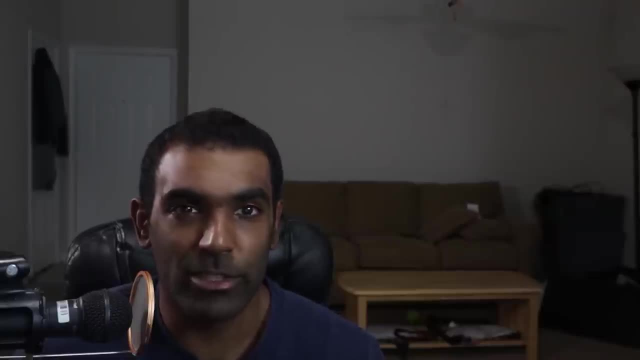 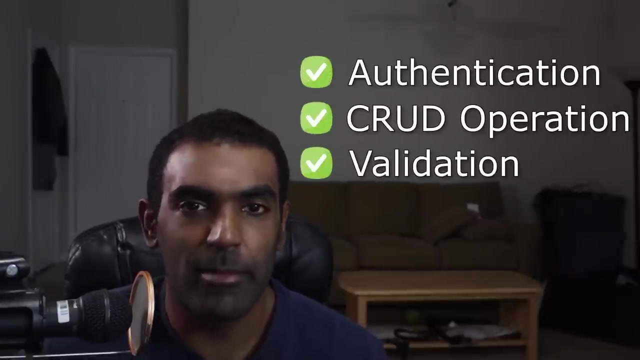 well, what exactly are we going to be covering for 19 hours? we don't need 19 hours to create an API. Well, first of all, we're going to build out a fully featured API that includes authentication, current operations, schema validation, and we're going to set up documentation for our API, because 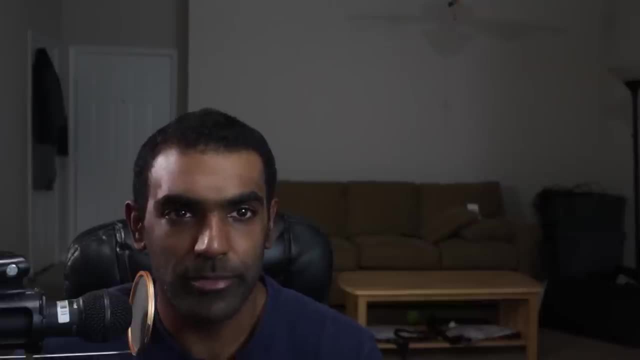 that's very important. However, the learning doesn't stop just there. This course is going to extend well past just basic API development. We'll also learn all of the tooling that surrounds building a complete and robust API. I've dedicated a large section of this course to learning SQL. 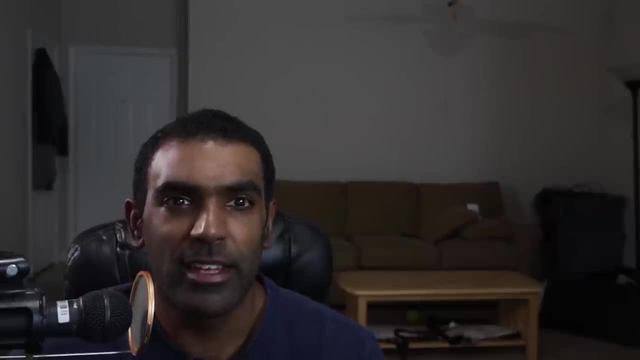 And I've noticed that a lot of the other API and web development courses. they just quickly gloss over SQL without diving into the nitty gritty of how SQL databases work. For this course we're going to cover SQL extensively And we're going to start from 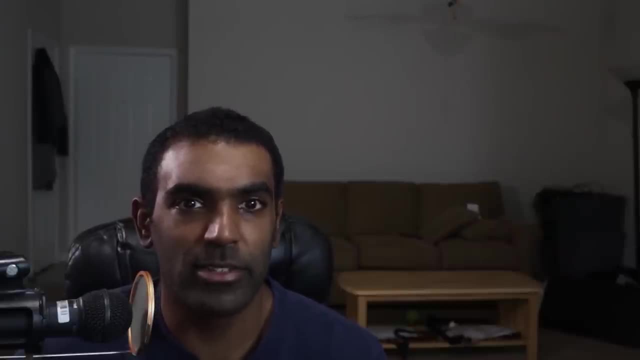 the absolute basics, So you don't need to know a single thing about databases or SQL in general, But by the time you complete this course, you will be very proficient at generating database schemas. you'll know core SQL concepts like primary keys, foreign keys, table constraints. 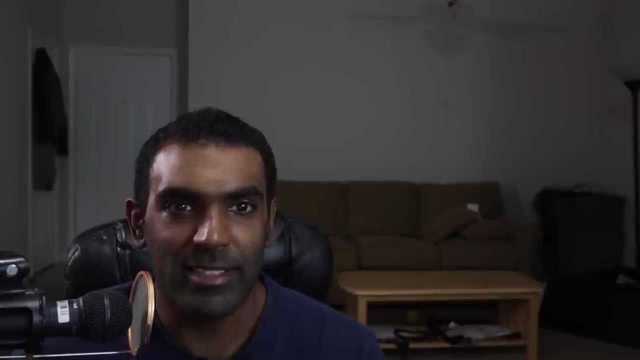 and you can pretty much be able to generate SQL queries to grab the exact data that you're looking for, And on top of that, I'll show you how to integrate your SQL databases in your API using two different methods, So we'll cover both, using raw SQL queries as well as ORMs. 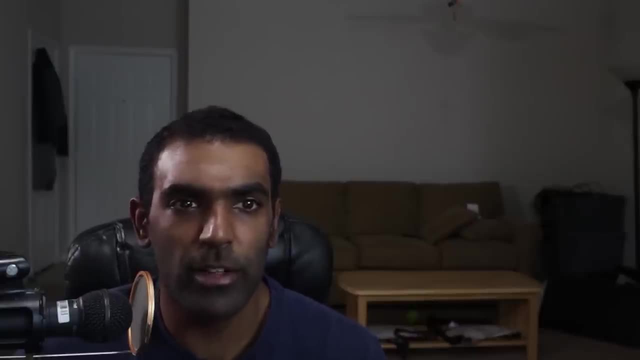 so that, no matter which method you ultimately prefer, you'll have all the skills and resources to start building out your own projects. We'll also familiarize ourselves with database migration tools like alembic, which allow us to make incremental changes to our database. 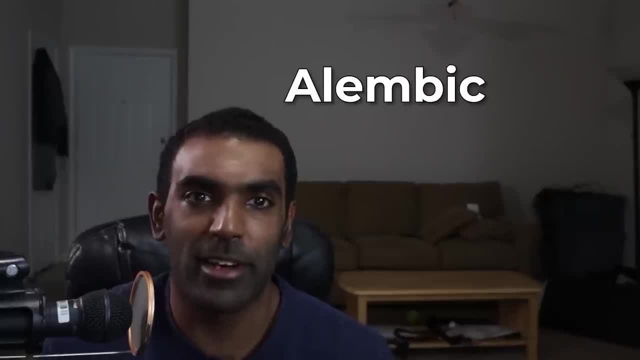 schema to track changes in Git, just like we can with our regular Python code. We'll also learn how to to use tools like postman to construct HTTP packets so that we could test our API during the whole development process. And when it comes to testing, I've added about, you know two to 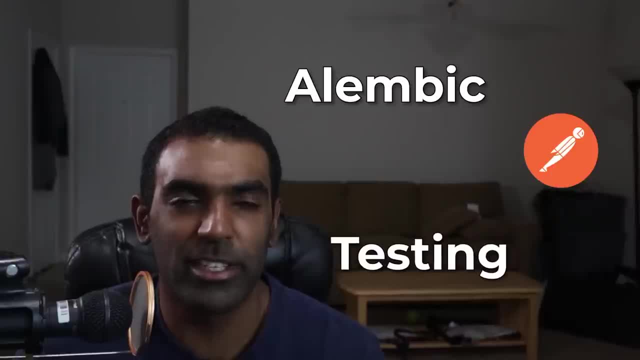 three hours of content going over how to set up automated integration tests so that, when you make changes to your code, you can run these automated tests to verify that your code changes haven't broke any pre existing functionality. And then, after testing, we're going to move on to the 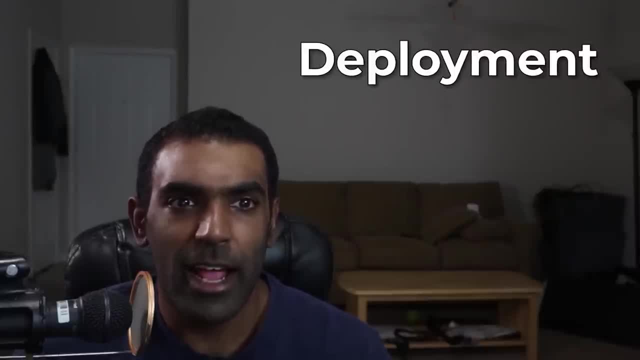 deployment phase. we're going to actually deploy our application, And I didn't just include one method of deployment. I've actually included two different deployment scenarios. The first scenario is probably the most common scenario, which is deploying our app onto like an Ubuntu. 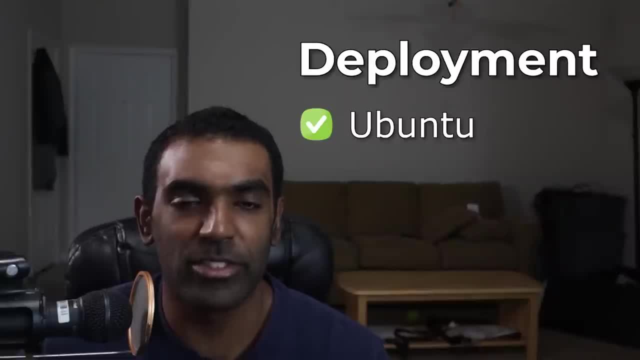 machine that can be hosted on any cloud provider like AWS, GCP, Azure or even DigitalOcean, And you know, we'll cover things like how to set up nginx to act as a reverse proxy. we'll we'll configure our own system D service, we'll set up a firewall to block all non HTTP traffic And we'll. 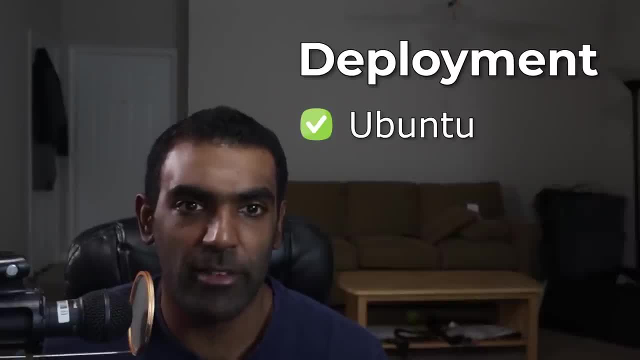 even set up SSL so that our application can handle HTTPS traffic. But after that we'll also take a look at how we can deploy our application onto Heroku, Just because, if you don't have, you know, maybe you can't afford to pay for cloud services, or you just don't have the ability to sign up for. 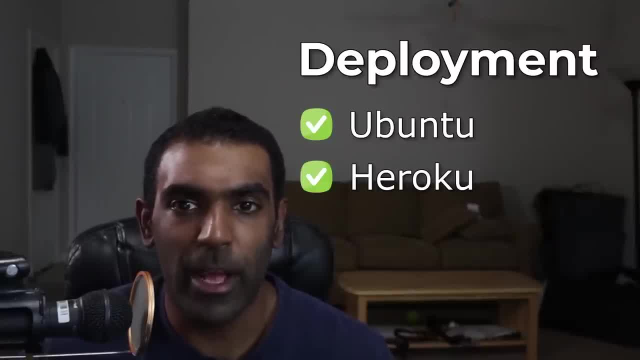 an account or something like that. I do want to make sure that you still have a way of deploying your applications, that you can show off to your friends and family what you created. So I added the Heroku section, because they've got a very, very nice and convenient free tier where we can. 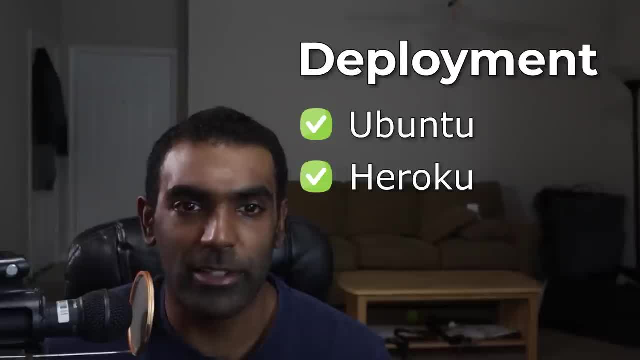 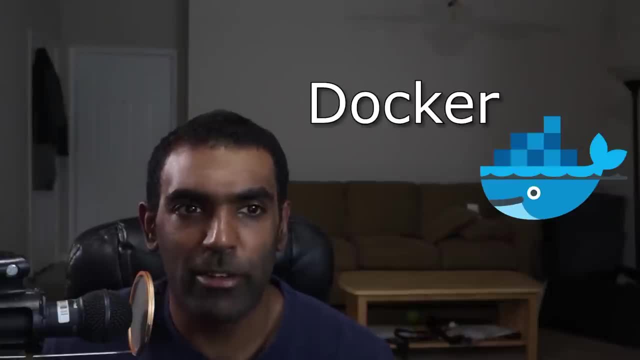 deploy our entire application for free. we don't need to sign up with a credit card. So that's why we're going to show you how to dockerize your API, in case that is your preferred method of deployment. And then, finally, we're going to wrap things up by building out our very own CI CD. 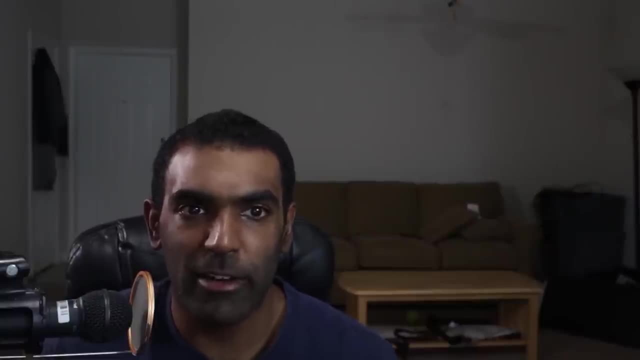 pipeline using GitHub actions. This will allow us to push out changes to GitHub resulting in our pipeline running, which will pull our code, run all of our integration tests, build all of the necessary images And, if all the tests ultimately pass, it'll actually push out our changes to our 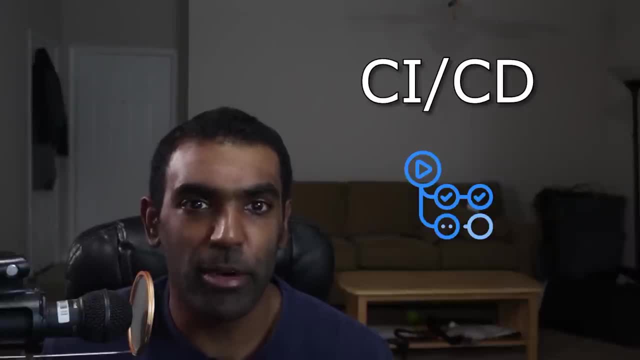 production environment so that we can do all of our integration tests, build all of the necessary images and, if all the tests ultimately pass, it'll actually push out our changes to our production environment. So we can do all of this in an automated fashion without having to manually go in. 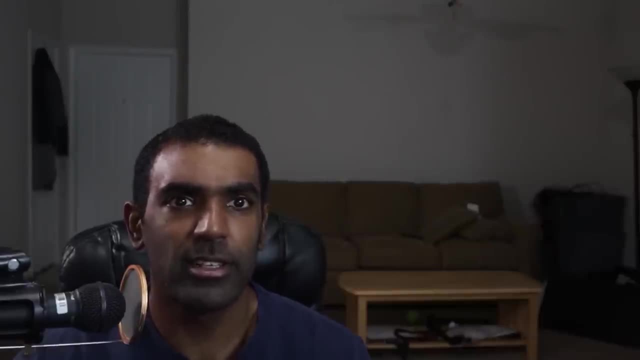 and run each step manually. So let's take a look at our tech stack. Since this is a Python API course, we will be using Python to build out our API. There were a couple of different web frameworks in Python that we could have used, most notably Django and flask. I decided to use neither one of them. 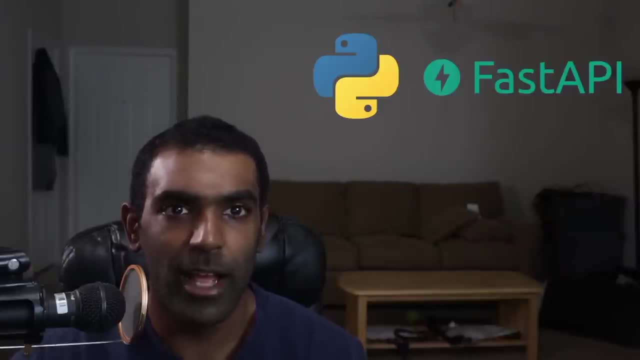 And I decided to use a newer framework called fast API, And the reason why I chose to use this framework was because it has APIs kind of built in mind. right, It wasn't there to address like the scenario. it really is all about building out APIs And on top of that it is really fast, right, But 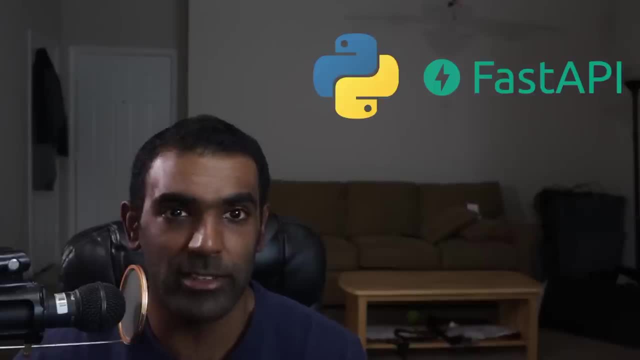 when I say fast, it's not just fast from a performance perspective, which it is, but it's also fast from the fact that it can. it makes it really easy and quick to spin up new APIs, And one of my favorite features of this framework is the auto documentation functionality When you build. 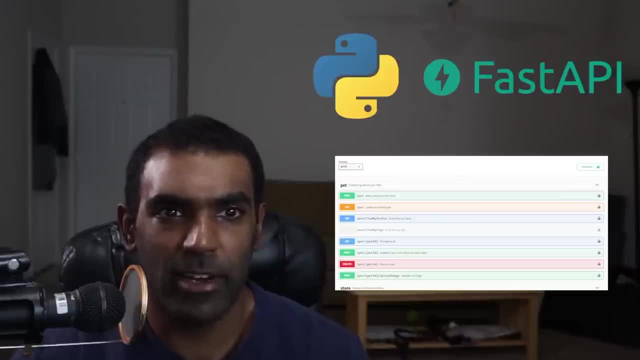 an API, you have to document how your API works, And this is a very cumbersome task, Because anytime you make any changes to your API, you have to remember to document how your API works, And so you have to be able to update your API, or then the front end can be making the wrong request fast. 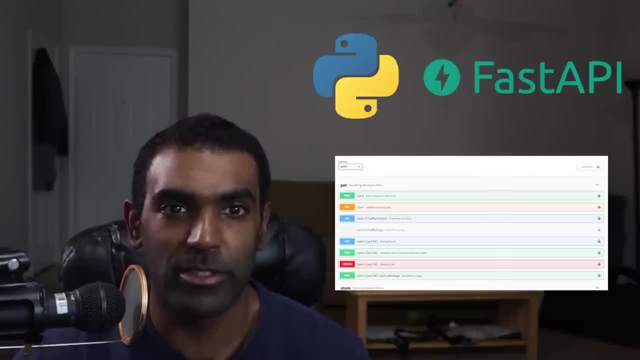 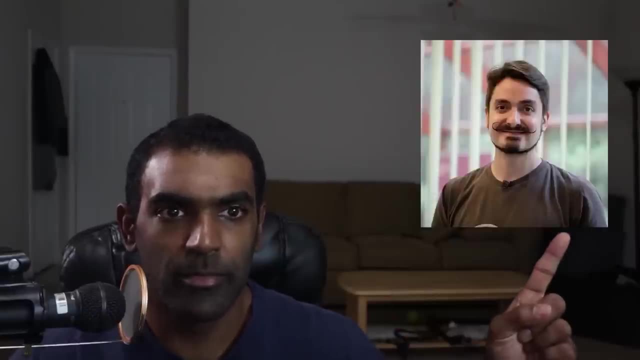 API automatically documents your API for you, so that you don't have to do it yourself. It's truly a game changer. And finally, the most important reason why I chose fast API is because of this. You see, this magnificent beast. This is the creator of the fast API framework And my mom. 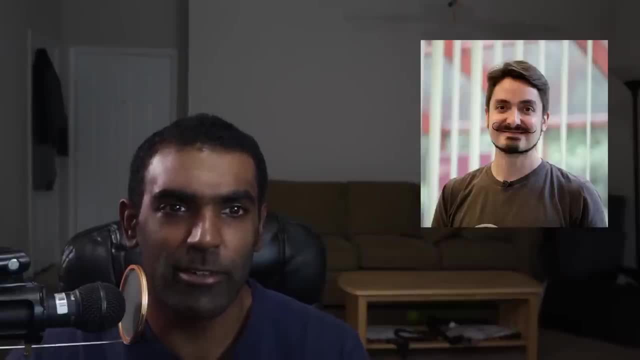 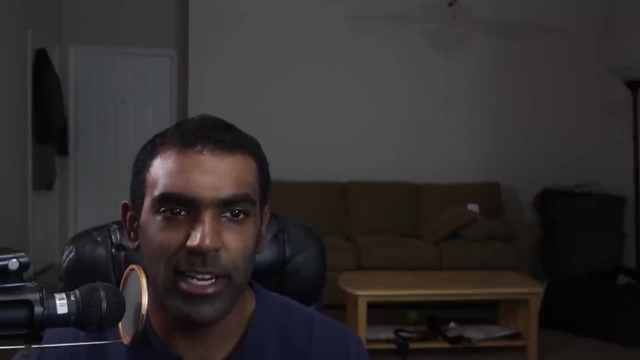 always told me: when someone with a mustache as glorious as that creates a web framework, you use that damn framework. Now, as I mentioned, we will be covering SQL extensively And I've decided to go with Postgres. It doesn't really matter what type of SQL database you use, They're all. 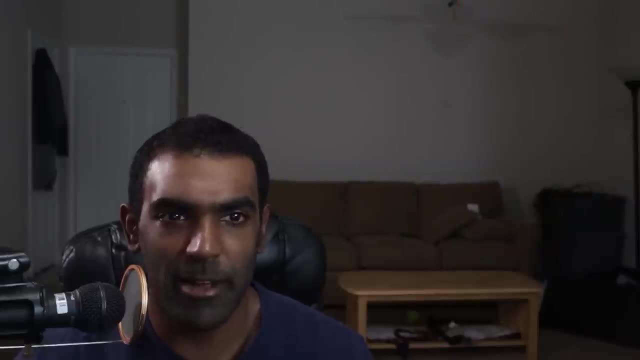 fundamentally the same, with only minor differences. I chose Postgres because that's my favorite- And who doesn't like elephants anyways, For our ORM. when we do eventually migrate to ORMs from using raw SQL queries, we will be using SQL alchemy. I decided to use that because that seems like that's. 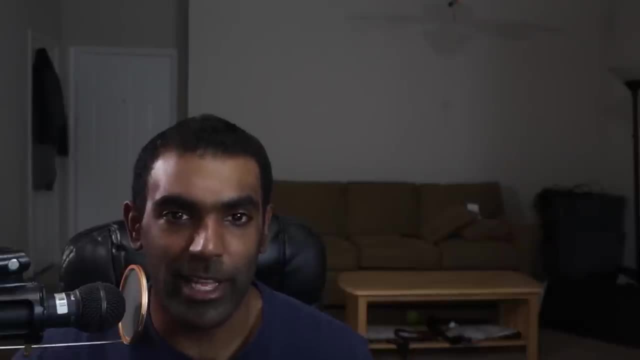 the most standard one for Python. I really could have chosen any of them. I didn't really care which one I used, So I just picked the most popular one. So that covers our tech stack. Let's now take a look at the project that will be coming up next. So let's take a look at the project that will be. 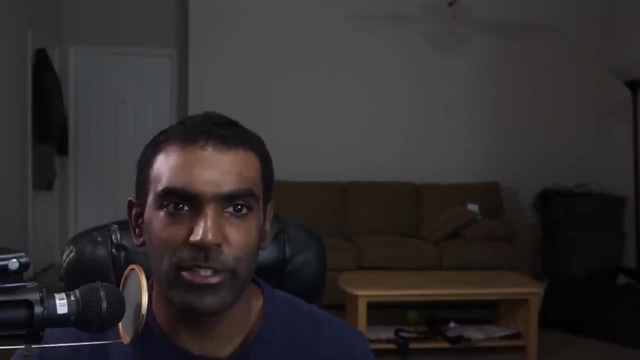 building. Now I would love to show you some cool, flashy website that you can show off to your friends. However, we're not building a website. we're building an API, And unfortunately, APIs don't really have a visual aspect to them, So I don't really have anything to show you, I mean, 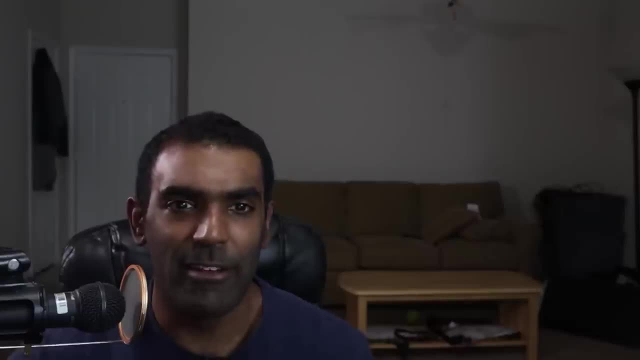 I could, I guess, construct a couple of HTTP packets and send it and verify that we get the proper JSON response, But that's not really exciting. So I'm going to do is I'm going to show you our documentation for our project, so that you can see all the different features that we 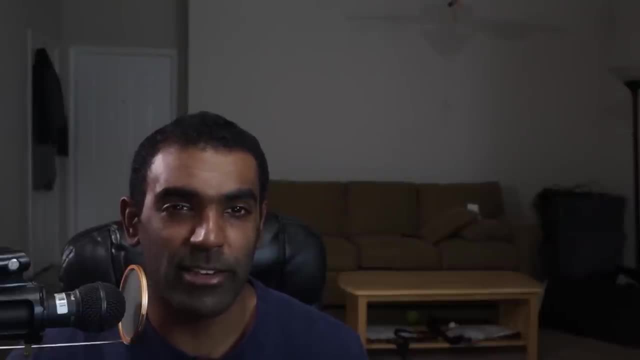 implement. And the nice part about the documentation is these are interactive docs, So from the documentation I can actually set up my own documentation. So I can actually set up my own HTTP requests to my application and get a response back. So you can really see all of the 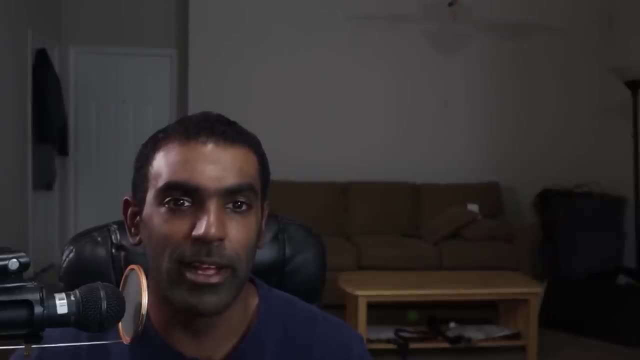 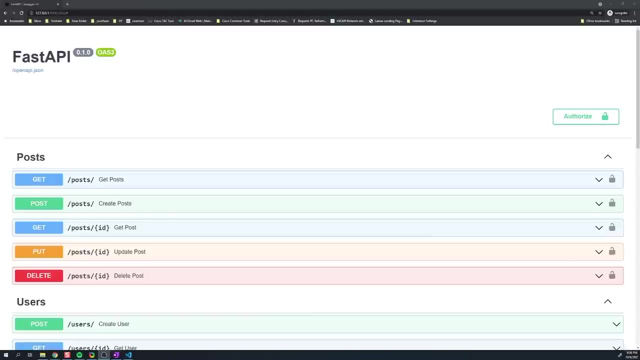 different features, things like the authentication and the crowd operations that we'll be performing and setting up in our API. So the app that we're going to build for this course is going to be a social media type application where users can create posts, they can read other people's posts. 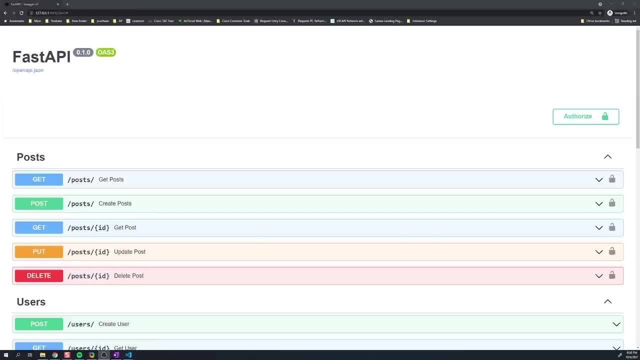 they'll be able to perform all the crowd operations, So they'll be able to create, read, update and delete posts, And we'll also be able to vote on posts. So you know, most social media apps have some sort of authentication, So I'm going to show you. 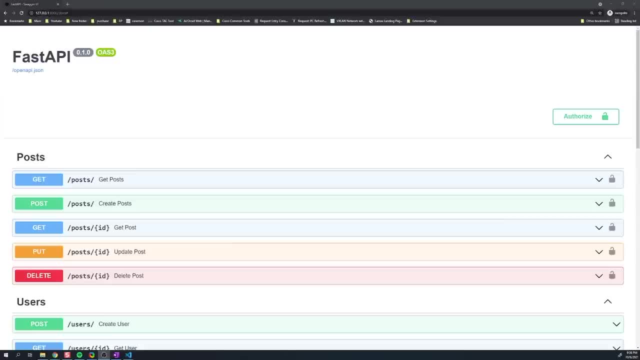 some sort of like system or voting system, And so we will be able to like other users posts as well. So this is the built in documentation that comes with fast API, And you'll be able to see all of the API endpoints that we're going to create in this course. So we're going to have 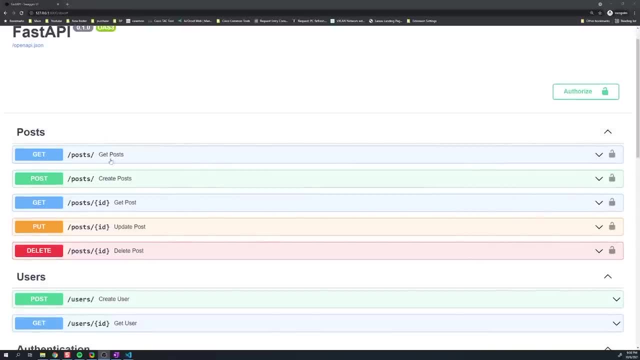 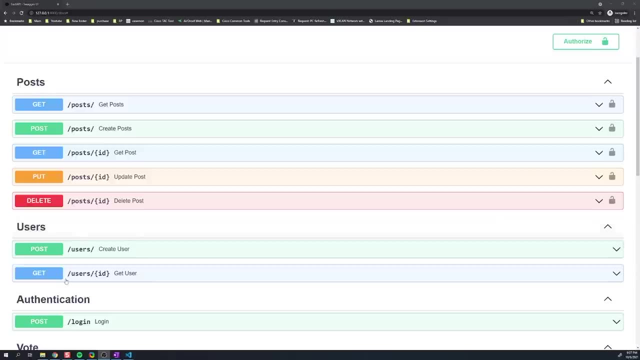 all of the posts endpoint, which is going to be responsible for retrieving all posts: creating posts, retrieving an individual post, updating a post as well as deleting a post. then we'll have the user specific endpoints of things like creating a user, getting a user's information. 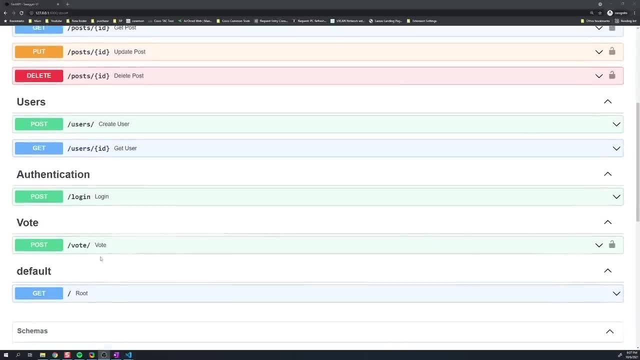 And then we've got our authentication, which is going to be used for logging in, And then, finally, we've got the one for voting. So when you want to vote on a specific, a specific post that you like, you can go ahead and like. 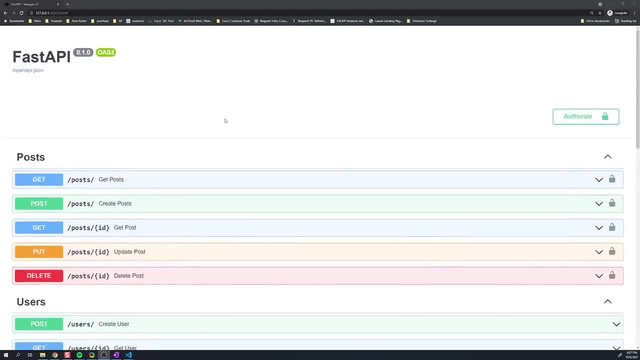 that post. So let's just use the documentation to actually, you know, test out our API. So, first things first, let's actually try to retrieve any or all of our posts. So if I hit this get button right here, we can actually try to send a request to our API with the built in documentation. So 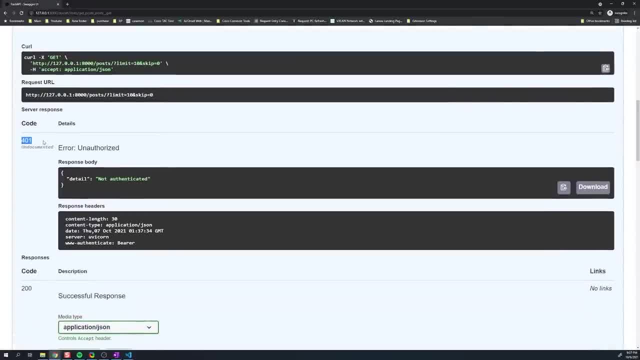 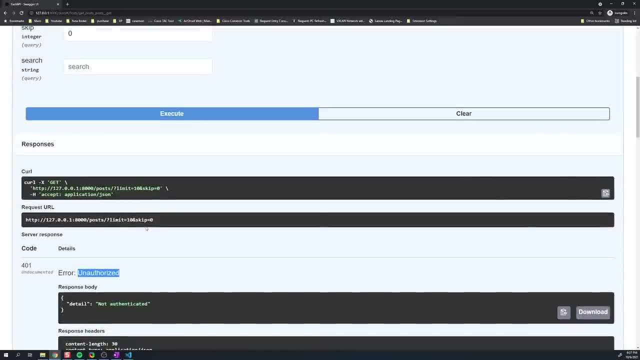 you can just say execute right and you'll see that we got a 401.. Which means that we are right now not logged in, So we are unauthorized to retrieve any of the posts. So the API that we're going to build is going to require all users to be logged in to be 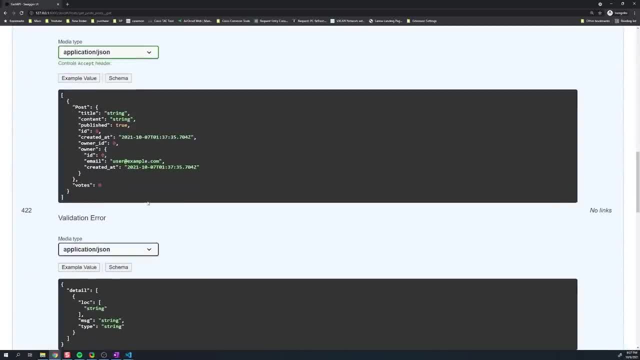 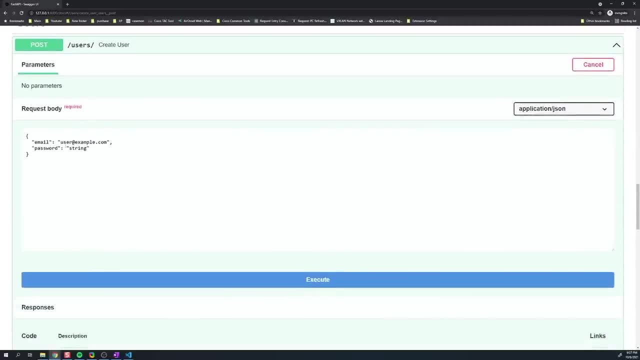 to even be able to read the posts. So let's actually go ahead and create a user And so we'll go down to the users endpoint under Create user, And I'm going to do try it out And it's going to give us an example of the structure of the data that we have to send to our API to create a user. 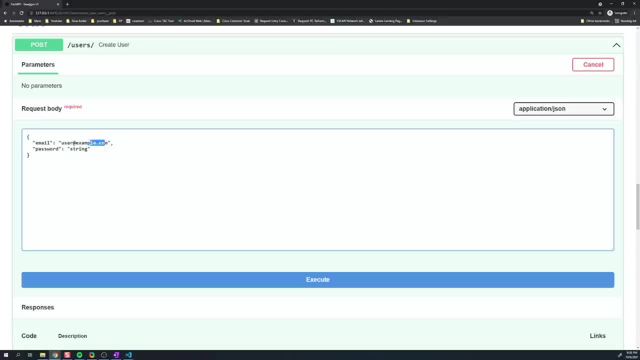 So we need to provide a username or an email and a password. So I'm going to create an email. I'll call this john On at gmailcom And the password is going to be something simple, just for demonstration purposes, And we'll execute that right. so it'll actually send that data back to our back end. you can see, we 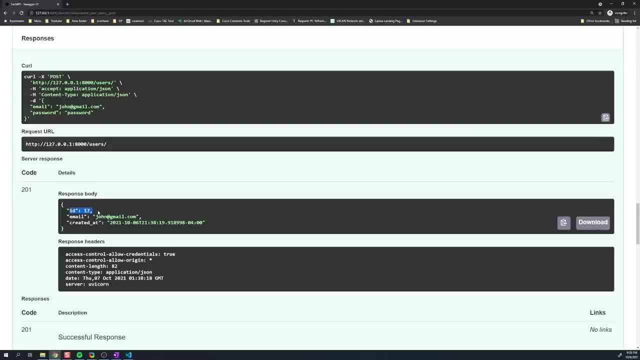 get a 201,, which means we were successfully able to create it. you can see the ID of the user account that was created. we can see the email is what it is, And then we can see the date that it was created at as well, And so now we can actually log in as this user. So there's a couple of different ways to 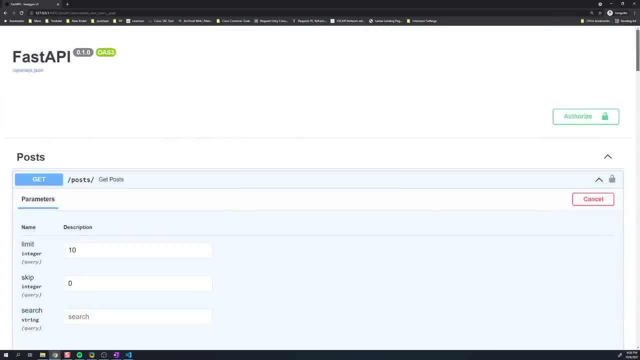 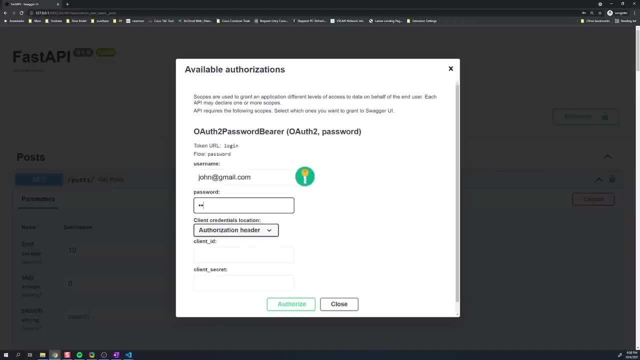 log in. I can go to the login endpoint or we can just go up here at the top and just do authorize And then we can provide that information. So I'll do john at gmailcom And we'll provide his password And if we do authorize now, 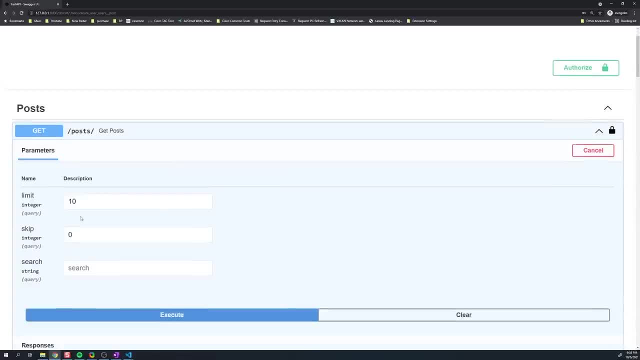 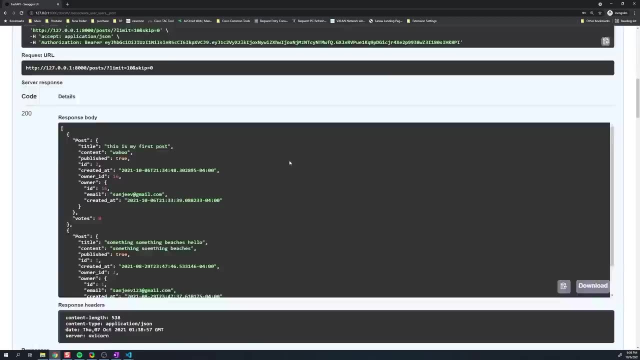 we can see that we have successfully logged in, So I'll close this out. And so now, if I try to retrieve the posts and then hit execute, you can see that we were able to retrieve all of the posts in our database. Right now there's only two, But you can see that these were created by some other. 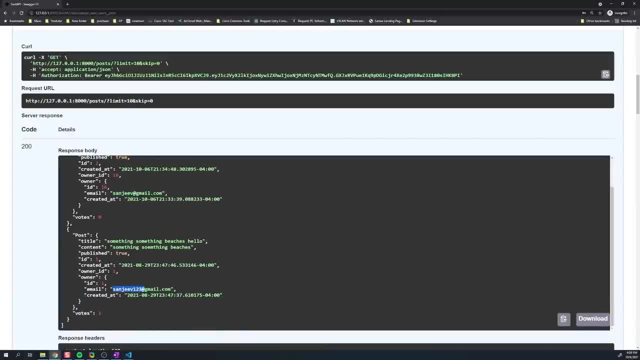 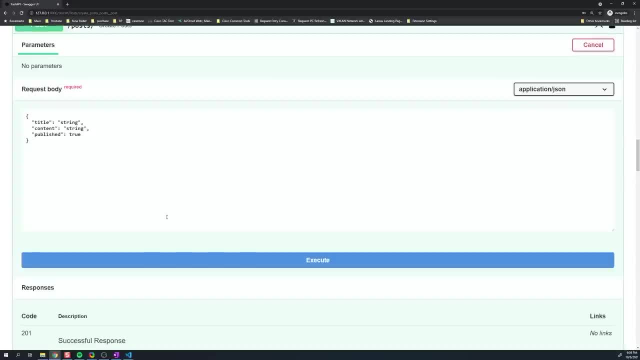 users like Sanjeev in this case, and then Sanjeev 123.. And if we want to create our own posts, we can go ahead and do that. So I'll go to the create post endpoint And we'll do try it out And it's going to give us an example here. So we have to provide. 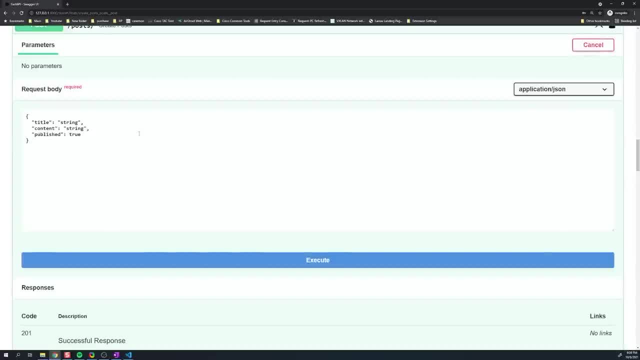 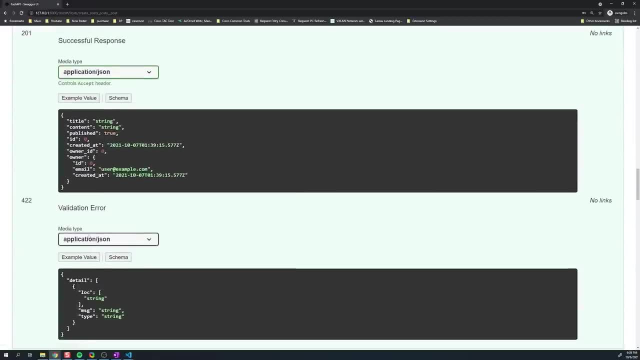 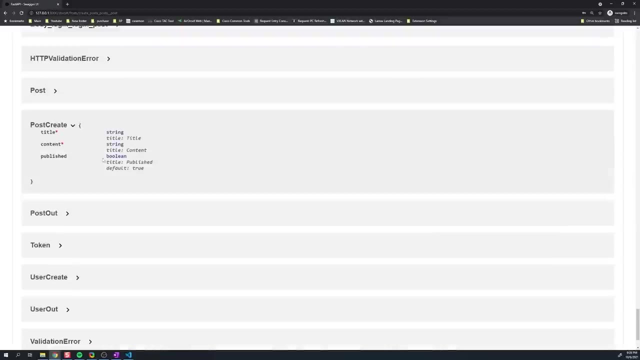 title content as well, as. is this post going to be published Or is it going to be a draft? And you'll actually see the structure of this schema Right down here. I think it's at the bottom actually. So if you go to post create here, this is going to show us the the schema. So if you go to post create, 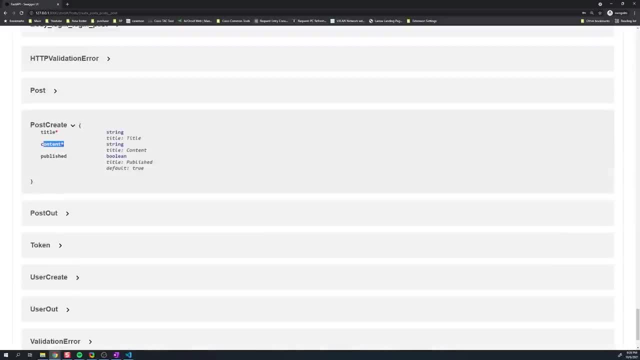 you'll see the schema that we have to pass. So we have to provide a title content. So this, the asterisk means it's required, the published is not required, And you can see that a defaults to true. So if we don't provide a value, it'll default to true. So let's test that out, And so I'll just say: 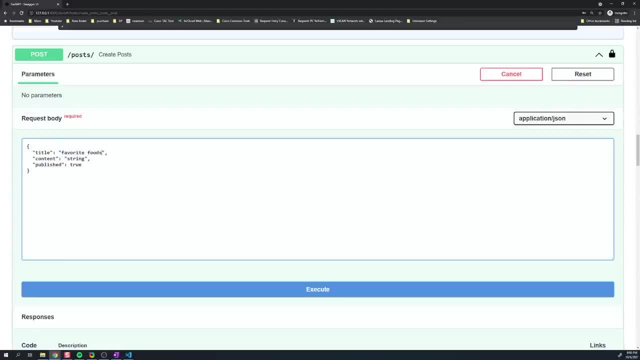 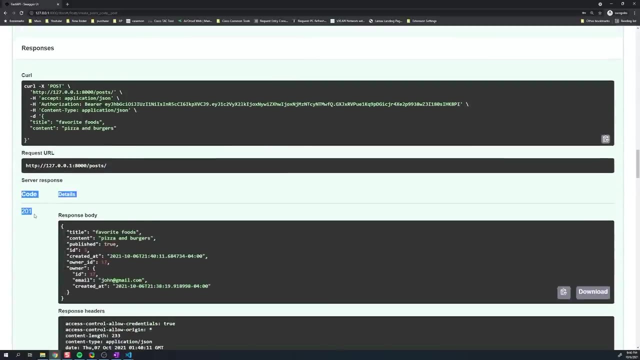 favorite foods is going to be the title And then content is going to be pizza and burgers And I will remove the published section because it is optional and no default to true anyways And we'll hit execute And if we take a look at the response, we get a 201, which means it successfully created it And 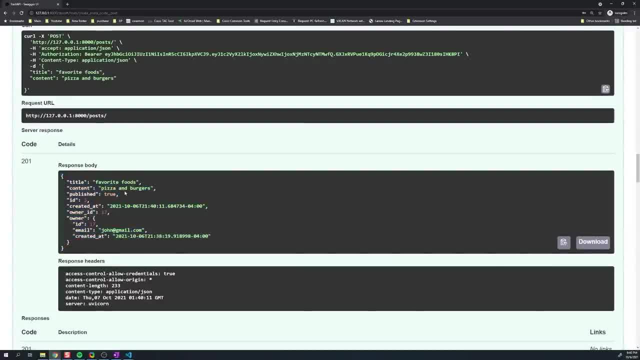 you can see what the post looks like in our database. You've got the title content. we can see the published got defaulted to true. we can see the ID of the post when it was created. we can see the owner ID, which is, you know who created the post, And so that's the ID of our account, which. 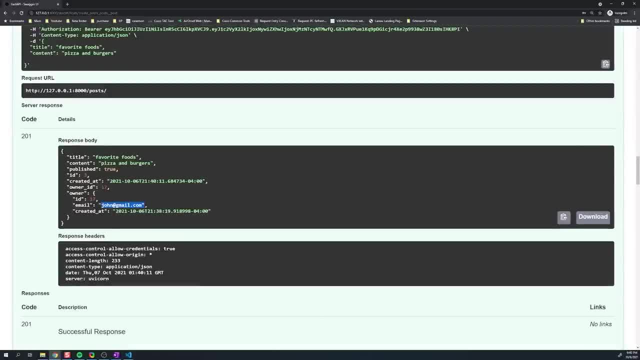 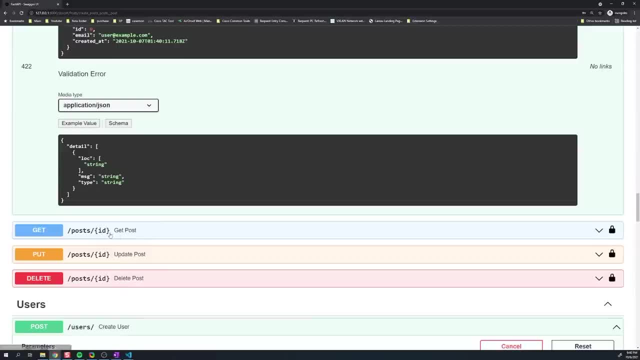 is 17.. And we can see the information about the owner. So this is john at gmailcom. And then you know, as usual, we can perform all perform all the other CRUD operations, So we can retrieve an individual post, update it and delete it. 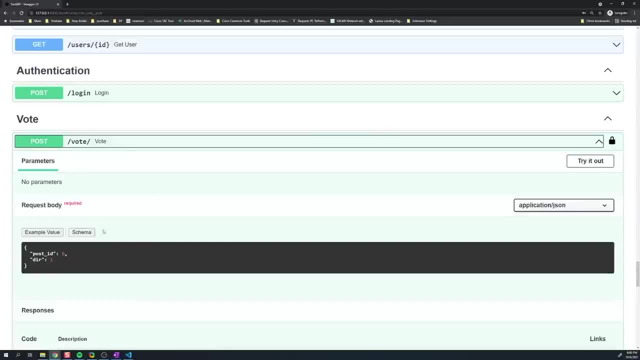 And then, once again, if we go down here, we can also vote to like a post as well, And so you know, this kind of forms the backbone of a traditional social media type application. So once you can really do this, you can really create any application you want, And I think this covers. 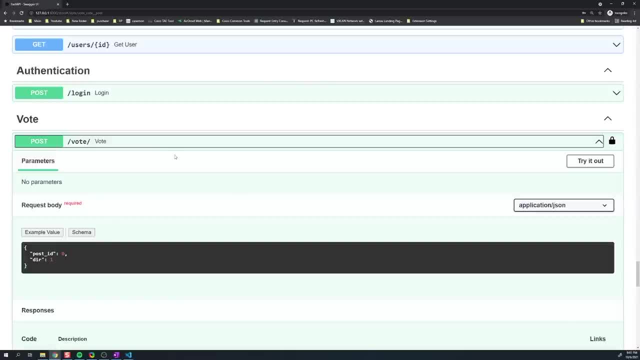 enough things from an API perspective, as well as from a SQL and database perspective, that you will have a solid foundation to really build out any API that you're interested in building out. And so I think that's enough talking. let's get to actually start coding out our application In this. 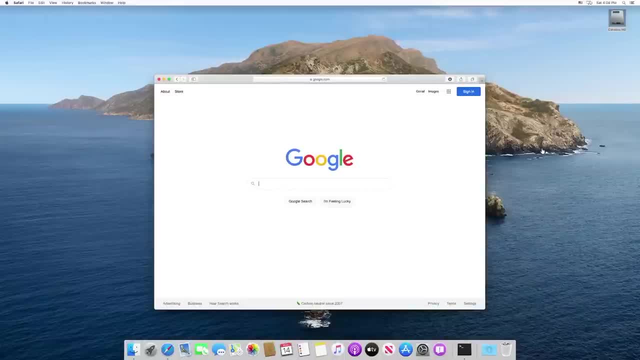 video we'll take a look at code and build our application at how to set up Python as well as VS code on a Mac machine. The first thing we're going to do is we're going to just search for Python And the first result should take us to the main Python. 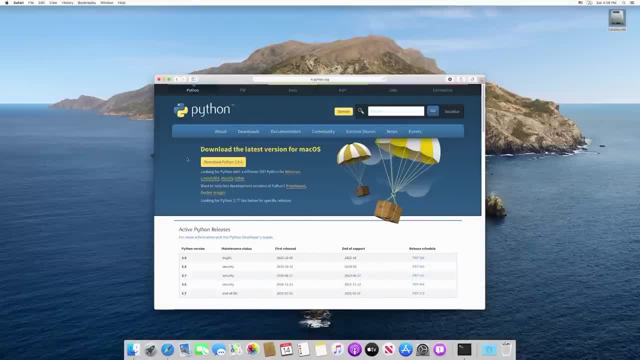 page And what we want to do is select downloads. It's automatically going to give us a button to download whatever the latest version of Python is, And the nice part is it automatically detect what platform you're using. So it'll know that we're on a Mac And right now it says that the latest 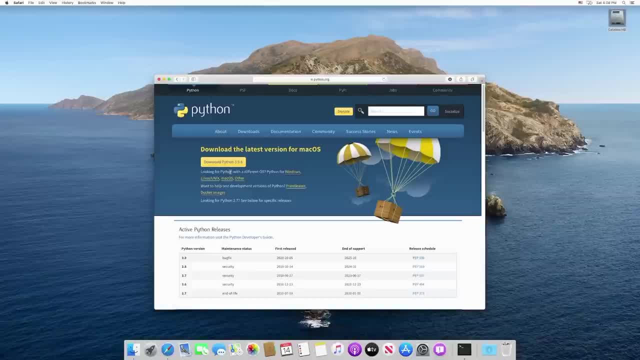 version of 3.9.6.. So it's going to offer me that. keep in mind if you're watching this video in the future, it's going to show a different version And it's okay for you to download a newer version. 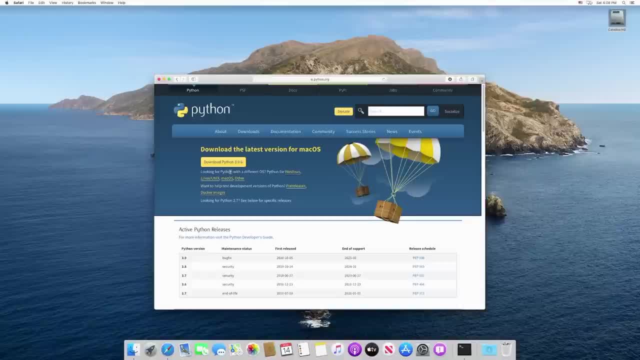 as long as it's later than 3.7, you should be okay for this course. So I'm gonna select this and it's going to download it like any other application. Once it's finished downloading, we're gonna select that and then select the file that we just downloaded, And then this is going. 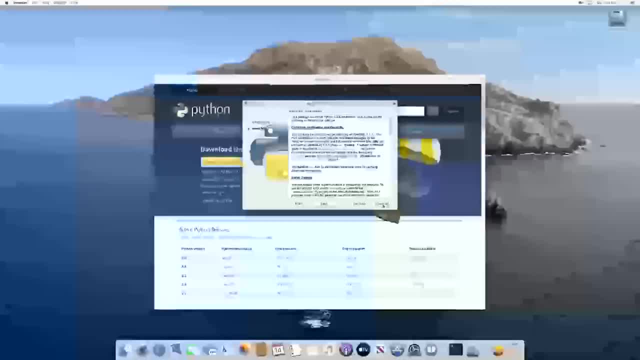 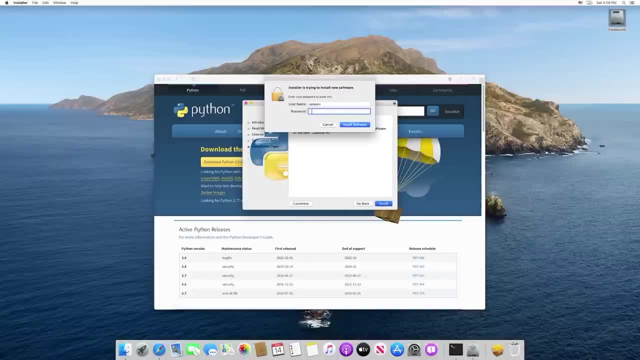 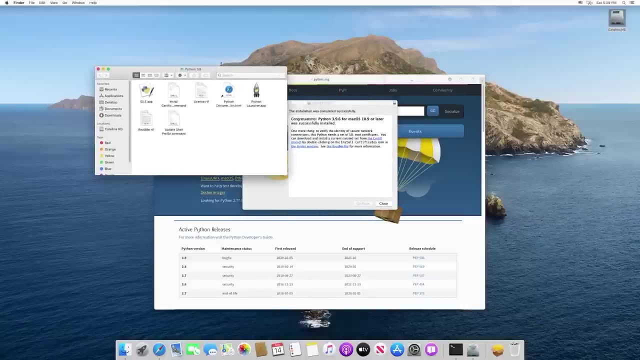 to take us through the Python installation process. So we'll hit continue, we'll hit continue, again continue. We'll hit agree And then install. And that's going to prompt us for a password. All right, and so once you get this pop up, it means that Python was successfully installed. 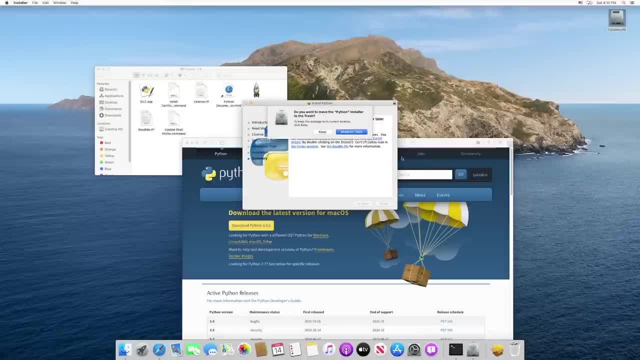 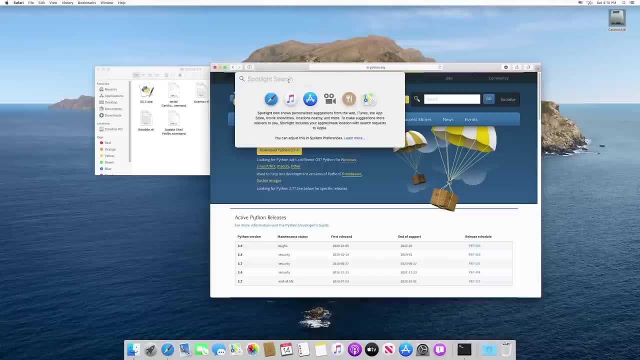 So we can then close that out real quick And then we can move this to trash. And the next thing that we want to do is go up to your search bar at the top And I want you to search for the terminal application And should find that. just double click on that So we can open up a terminal. 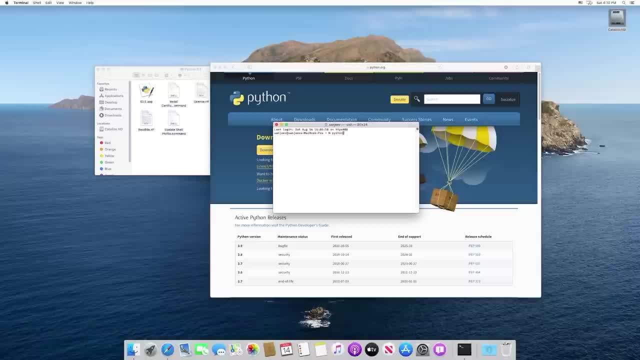 And with our terminal. what we want to do is we want to type in Python three dash, dash version, And the reason we specify Python three is that you can actually have a Python two and a Python three version simultaneously installed simultaneously on your machine. we want to make sure that we got Python three successfully. 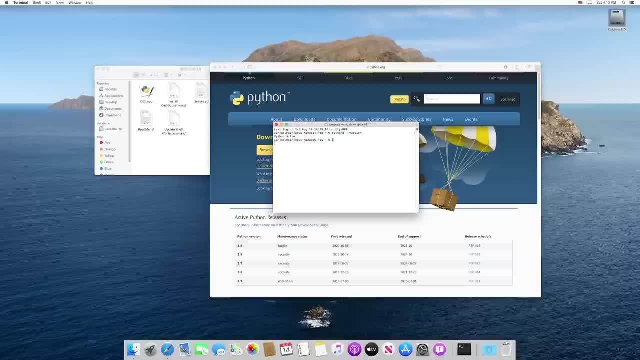 installed. So if we type this in, it should then print out the version that we installed, So we can see that we did successfully install Python three, dot nine, dot six. So we should be set from a Python perspective And now that we have Python installed, let's go ahead and install VS code. So, like I said, 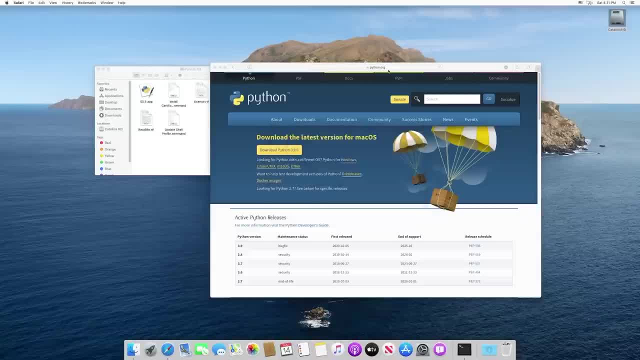 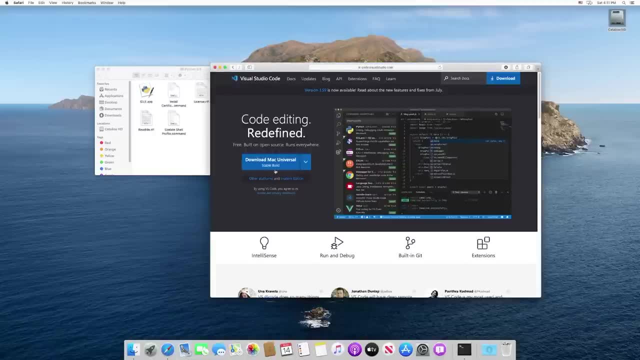 this is going to act as our text editor, or IDE, And so what we're going to do is just search for VS code, And this is going to take us to the Microsoft page, And then, once again, Microsoft will automatically detect that we're running a Mac, And then we can just go ahead and select. 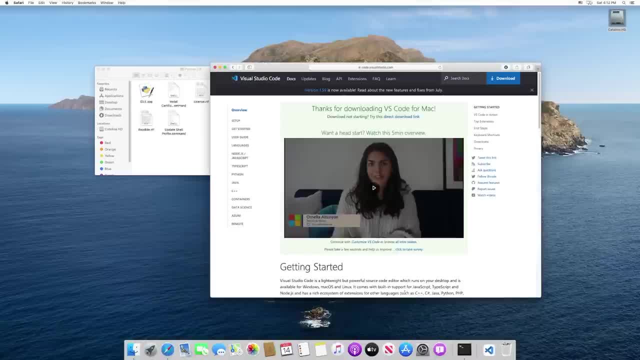 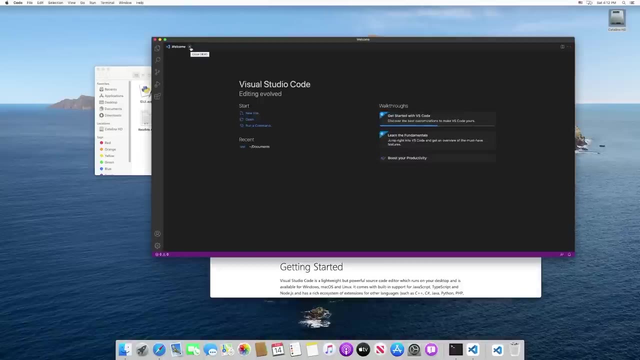 download Mac Universal. All right, and once that's done- installing or downloading- we can select that and open it up, And you'll get this warning: just go ahead and select open. And so this is going to be the default version of VS code And what we need to do is VS code is just a very basic text. 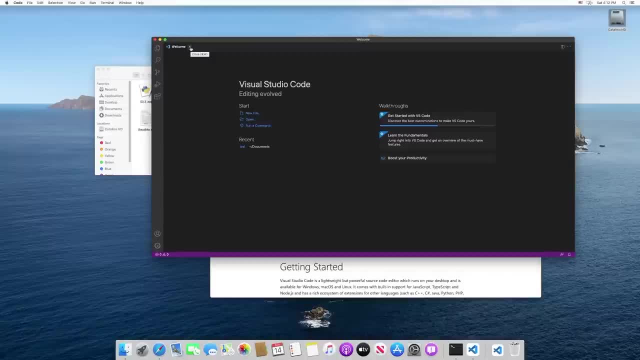 editor. However, it comes with extensions that we can install that make it significantly more feature rich, So it'll almost act like a traditional IDE And if you select the extensions icon, which is this icon right here with the extra blocks, select that and I want you to search for. 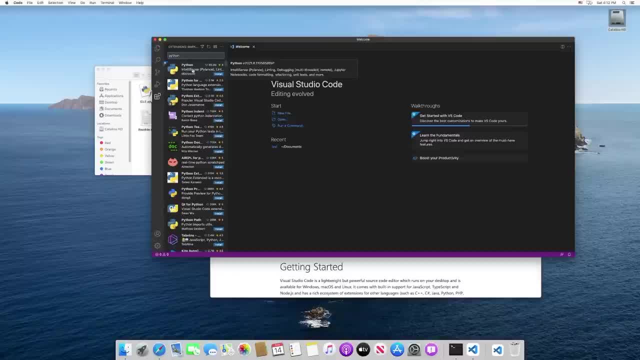 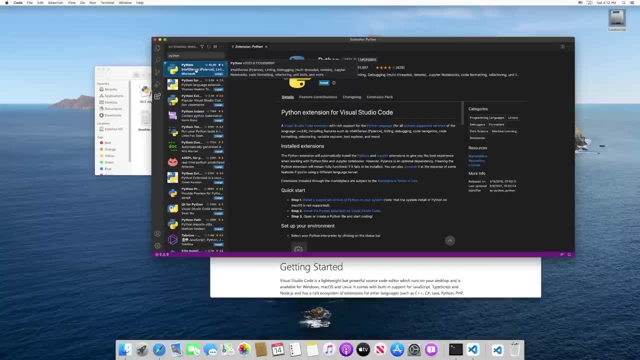 Python, And the first result should be the one you want and should be the one that's made by Microsoft. So this is going to provide things like linting, IntelliSense debugging and a few other features that are going to come in handy when it comes to writing Python code within VS code. 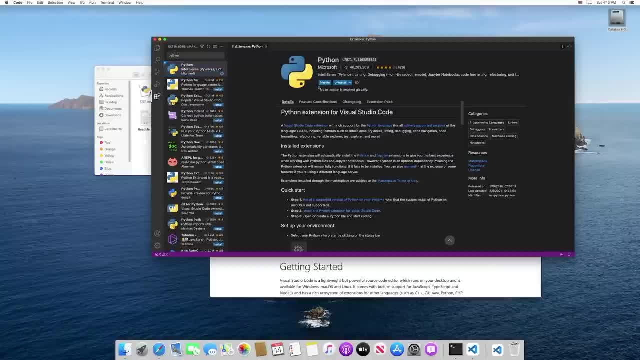 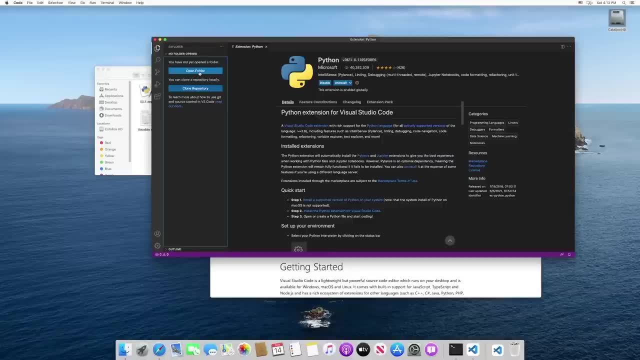 So go ahead and install this. Alright. so now that it's installed, what we want to do is like this icon to go back to our folder menu, And we want to select open folder. So what we're going to do is we're going to create a folder to store all of our project code. I'm going to select open folder Now. 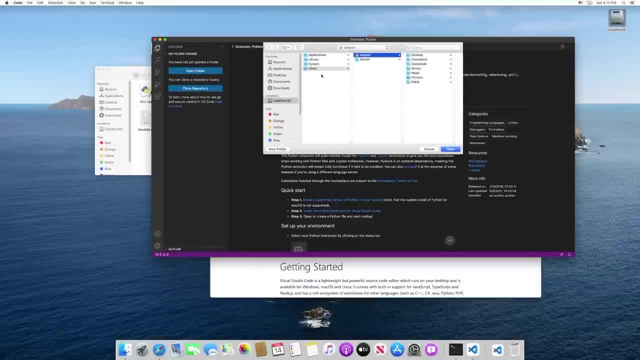 we haven't created a folder to actually store our application, So I'm going to go under my traditional users, Sanjeev, and then I'm just going to store this within my documents. I'm gonna make this a folder. I'll call this, we'll just call this fast API. I'll create that and then we're. 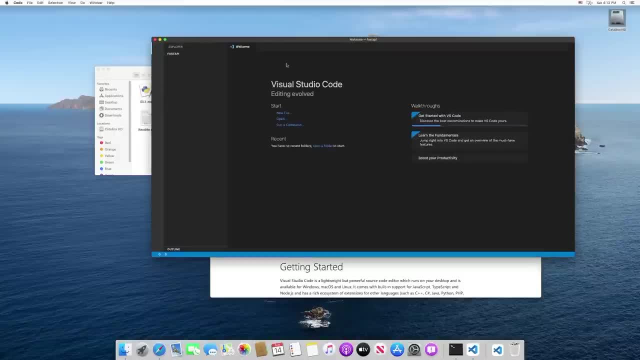 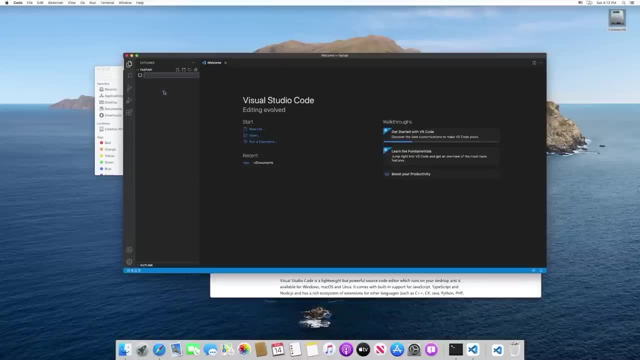 going to open up the fast API folder that we just created, And so this is going to open up all of our project code. right now we have no files, and that's to be expected, But what I want to do is I want to right click here and select new file, And we want to do is type in main dot, p, y And before we hit, 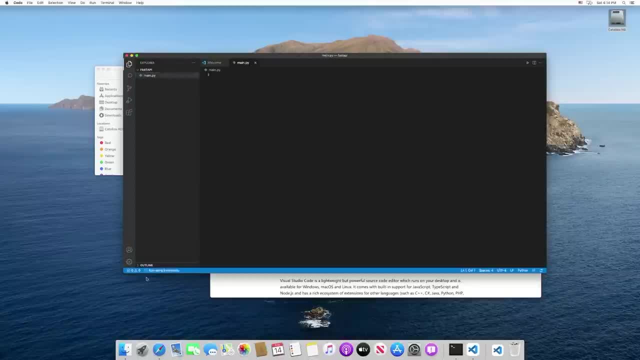 enter. I want you to look down here. So when I hit enter, you'll see that something's happening. So I'm going to go to the Python extension and it's automatically going to select a Python interpreter And so, like I said, you can have multiple different versions of Python. So 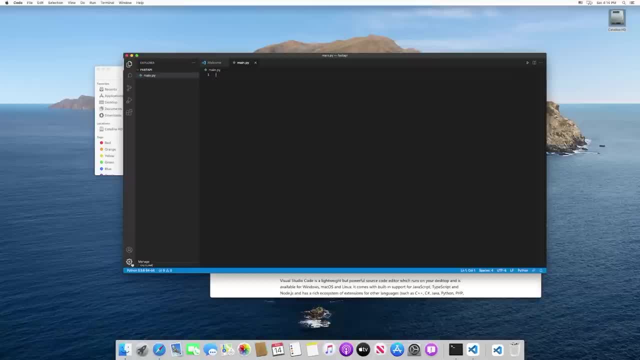 technically we could you know for any one of our projects. we can be running 3.9 dot six, or maybe we're running 2.7.. If we want to stick to Python two, we can actually select which specific. 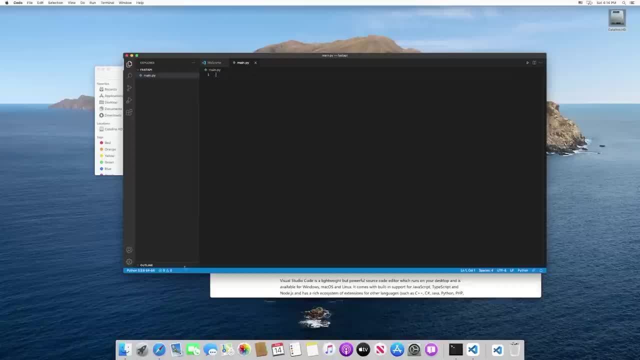 Python interpreter. we want to run on a per project basis, And if you ever want to change this- or for some reason it wasn't able to find this correctly- just go ahead and select View Command Palette And then it automatically found the most recently used ones, But you would just search for Python. 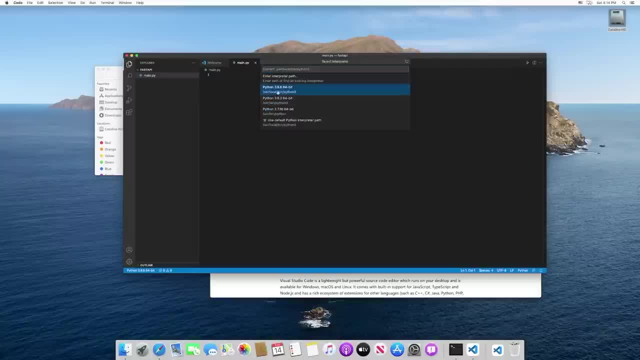 select interpreter. select this And it shows the currently selected interpreter. But you can also enter in the path to find a specific interpreter. So you would just find wherever Python 2.7 was installed. If you wanted to use that, or if it was unable to find 3.9 dot six, go ahead and just. 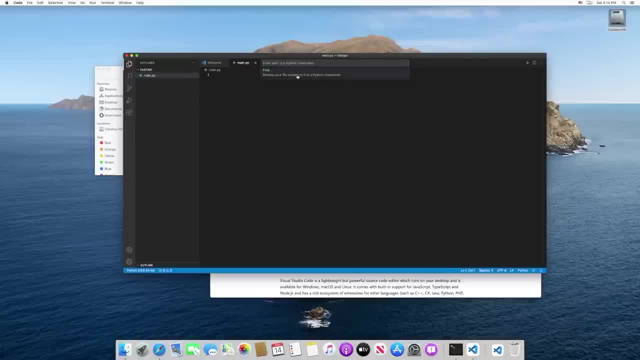 find where Python 3.9 to six was installed on your machine and point to that Python dot exe file. Actually, it's not called dot exe within Mac. I forget what it's called on a Mac. I actually use a Windows machine for most of my things. But that's all you have to do. 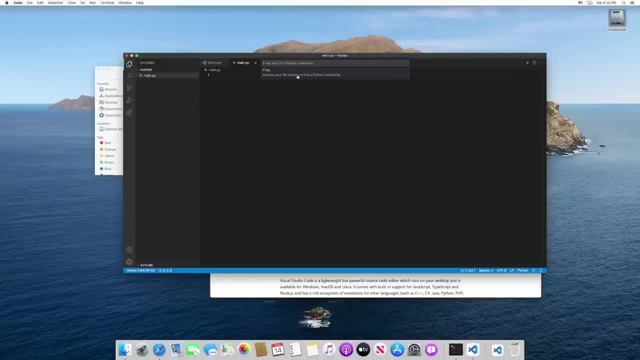 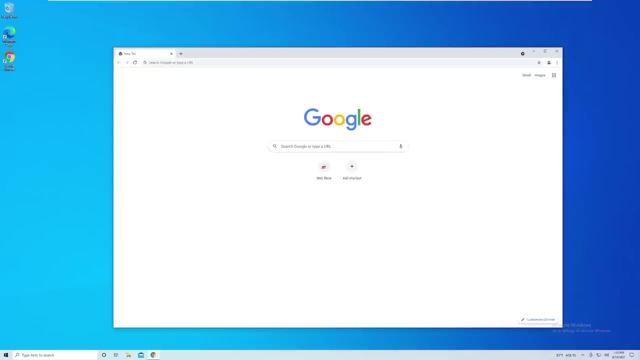 And so at this point we've got Python setup And then we've got our VS code setup. So, once again, anytime VS code closes, you want to open it back up, and then open up the folder fast API, in this case. In this video, I'm going to walk you through setting up Python as well as VS code on a Windows. 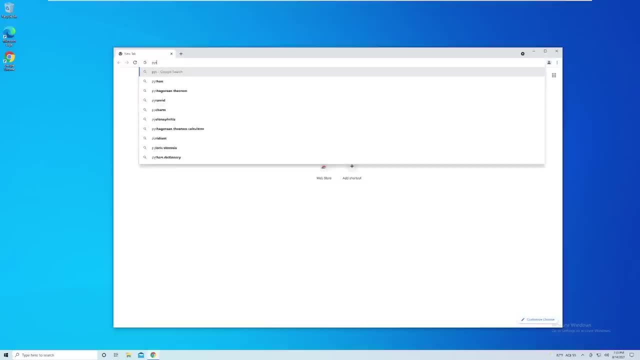 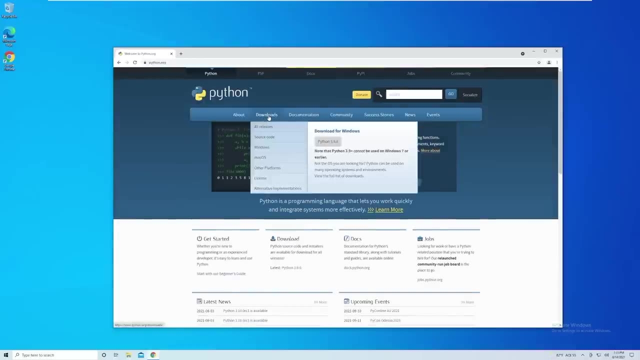 machine. So the first thing that we're going to do is, within your web browser, just search for Python, And then we're going to select the first result. So this is going to take us to the main Python page, And we want to go to the download section, And so here, Python the website is going to offer. 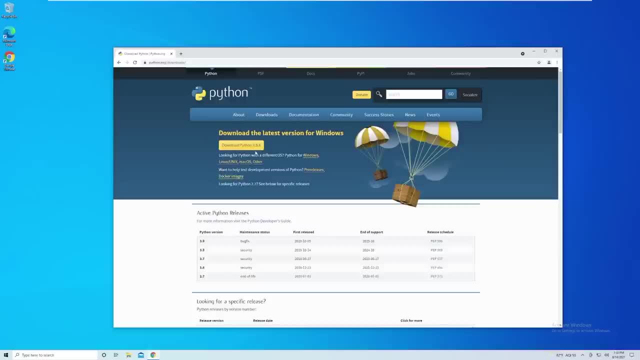 you up whatever the latest version of Python is. In this case it happens to be 3.9, dot six. Keep in mind, if you're watching this video in the future it's going to show some other version. That's okay. go ahead and just download the latest version, As long as it's a later than 3.7,. 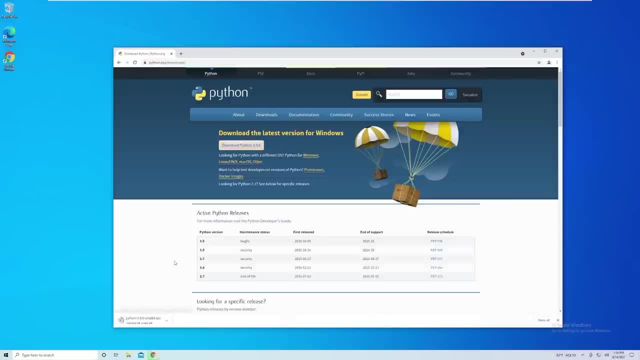 you should be okay. So I'm going to just hit download Python 3.9 at six. going to download that. once it's finished downloading, I'm going to select that and it's going to open up the installer. Now, with this installer open, it's very important that you select add. 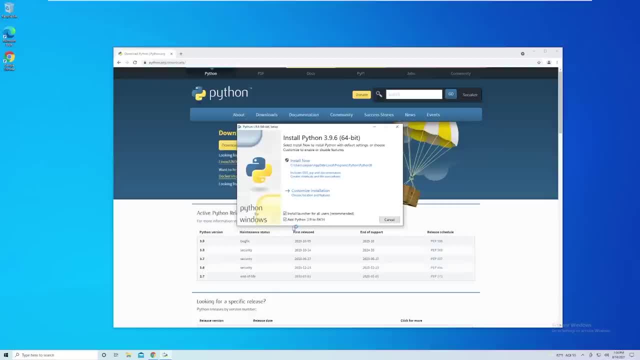 Python 3.9 to path. do not forget to do this, or then you're going to run into some issues. So make sure that's selected and then hit install. Now, if you go through the installation process and you realize you forgot to do this, technically, there's a way to fix it afterwards. But 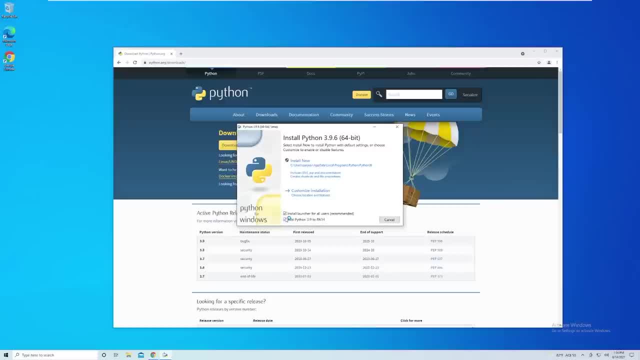 instead of me explaining to do that, the best thing to do is just uninstall Python and reinstall it, So we'll hit install. Now you'll get a pop up. just go ahead and hit Yes, Alright, and once you see this message where it says setup was successful, that means Python was installed. 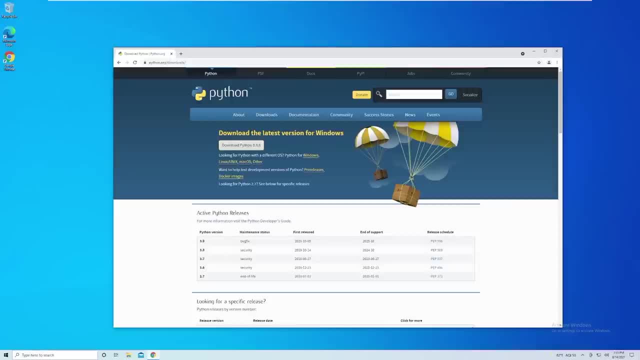 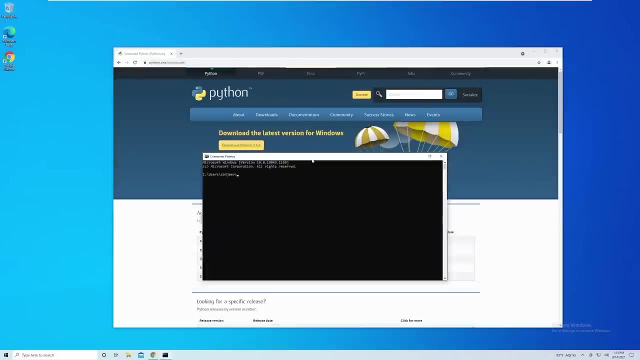 And the next thing that we want to do is just quickly verify that Python is up and running and working. So what we're going to do is we're just going to search for CMD, So it's going to open up our command prompt or terminal, And then in here, just type in Python: dash, three, dash, dash. 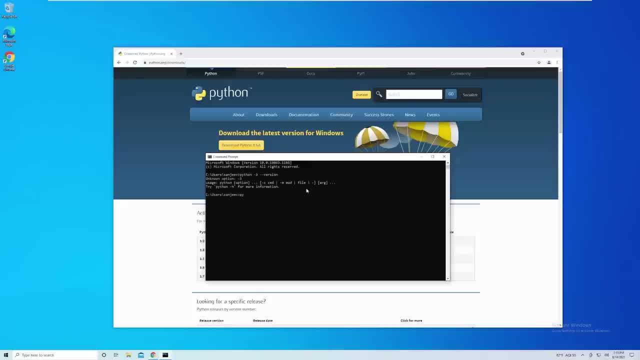 version. Sorry, we should actually type in Python py dash three, dash, dash version. Alright, and so when you type this command in, it's going to tell us the specific version of the version that we're going to install, So we can see that I was successfully installed. Python three, dot nine, dot six. 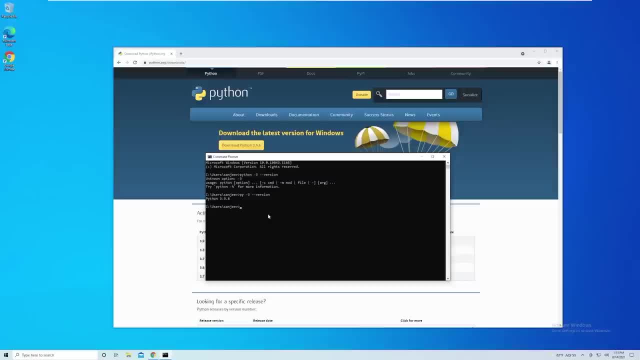 if you get any kind of error or any message saying that this command is not available, that means that Python wasn't installed successfully. So just go ahead and redo that process, just in case. Now the next thing that we want to do is install VS code, So let's. 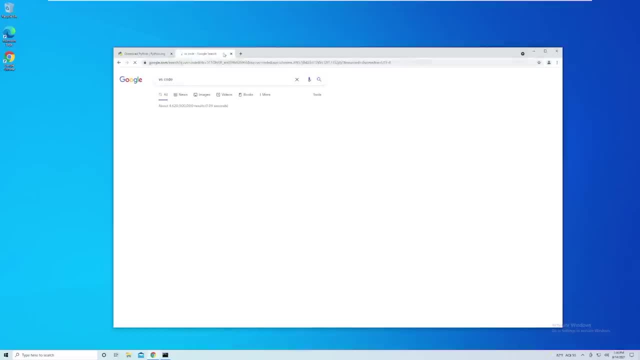 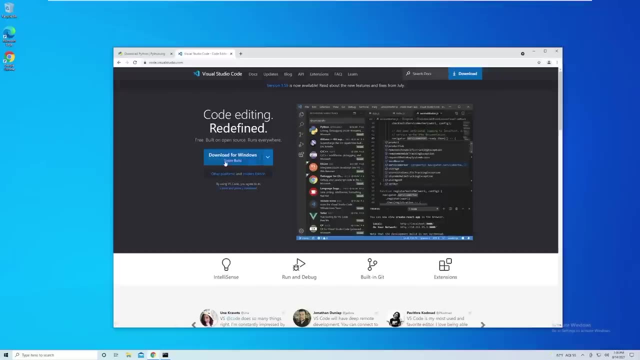 open up a new tab, just search for VS code And then we'll select. this is going to take us to this page And you'll see that a VS code will automatically detect what version you're running, So you can just like download for Windows. 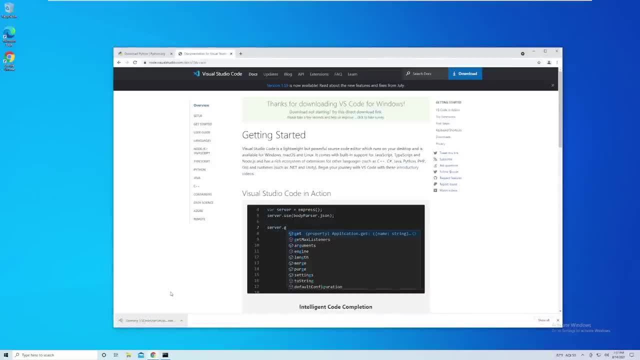 And then, once it's finished downloading, go ahead and open it up, Hit the accept agreement, hit next, next, next, And then you can leave everything as default And then go ahead and run. install All right and then go ahead and finish. 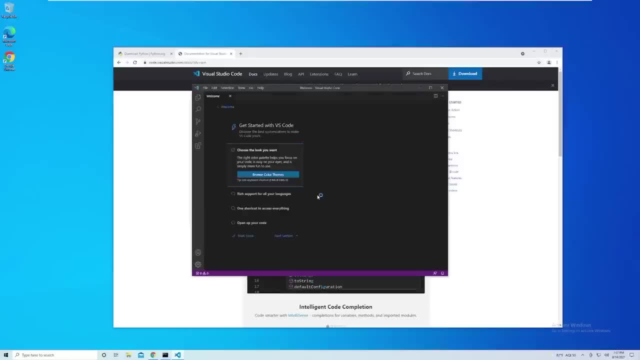 it's going to automatically open up VS code. Now there's a couple things I want to do. So VS code, at its core, is just a basic text editor. However, we can install extensions. they give it extra functionality, extra features that will make it operate a little bit more like. 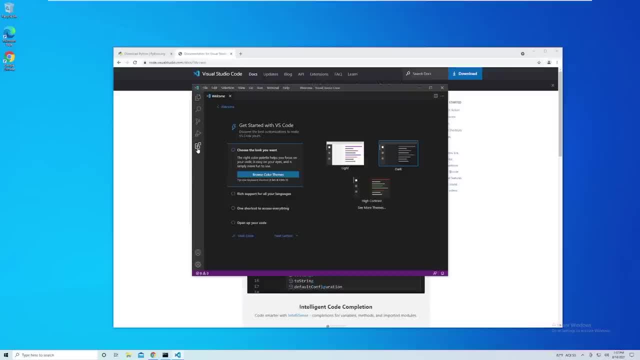 a full blown IDE. So go ahead and select this icon right here. This is for extensions. And then what we want to do is we want to search for Python, And we usually just want to select the first one. it'll have a star and it's gonna be the one made by Microsoft. you'll see that there's other ones. 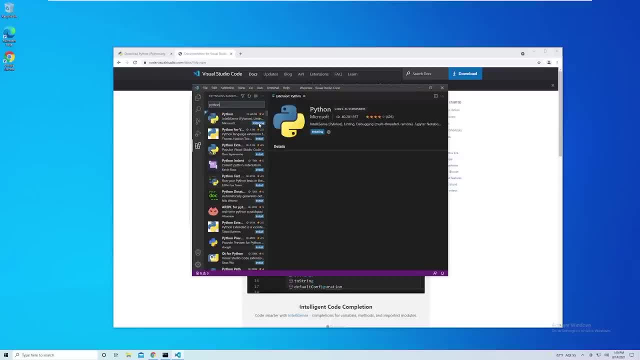 made by other users, but we want the main Microsoft one hit install, And so this extension is going to give us IntelliSense, linting, debugging and a few other features that are going to make it a little bit easier. So we're going to go ahead and install it And then we're going to 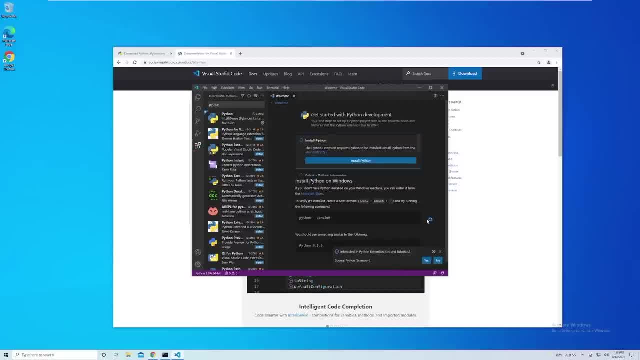 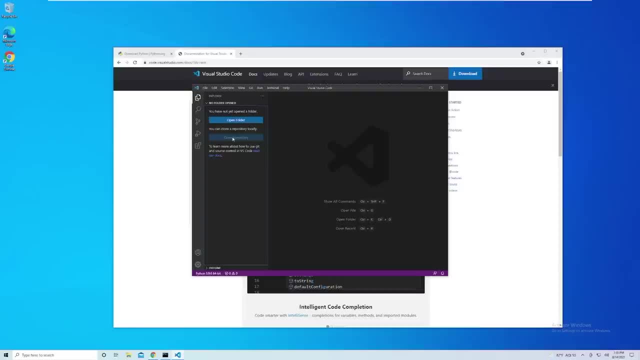 start working with Python within VS code. Alright, and so now that it's done installing, we can just close this, close this and then select this one to get back to your main file browser. And right now we haven't opened up any folder. So what we want to do is we want to create. 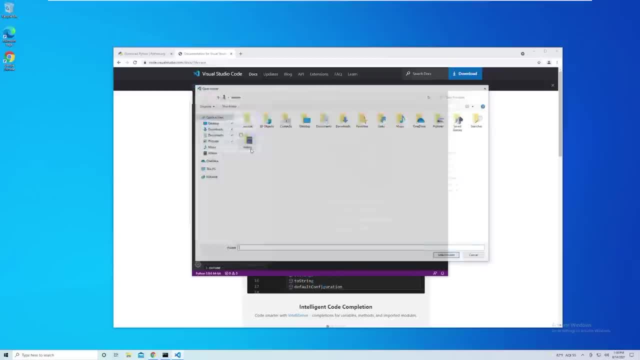 a folder to store all of our application code. So select open folder and then figure out where you want to store your application code. So I'm just gonna store this in my documents. you can store this wherever you want. I'm going to create a new file or a new folder. I'm just gonna call it fast. 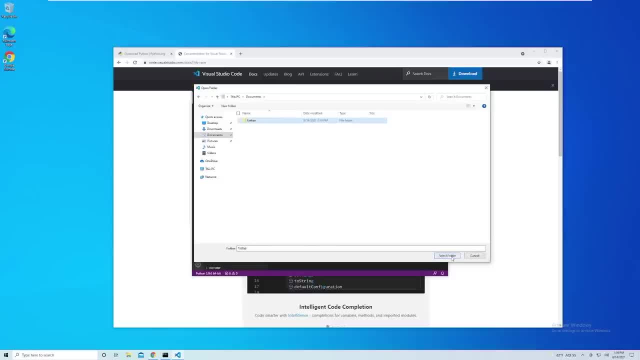 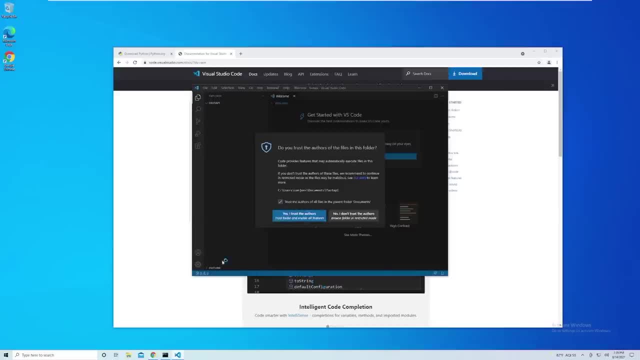 file, But you can name your project whatever you want. So just select folder And so that's going to not only create, not only create the folder, but it's going to open it up within VS code. If you get this error, just like trust the author And just like yes, And then we can close out this. 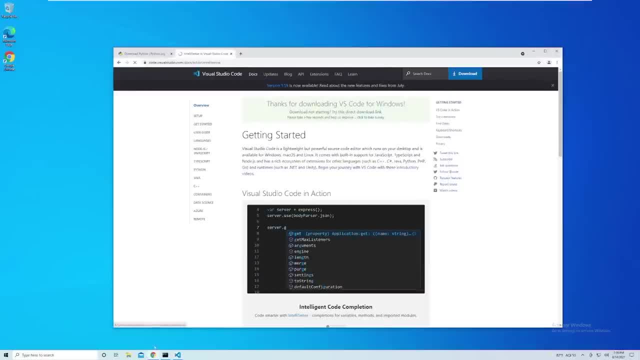 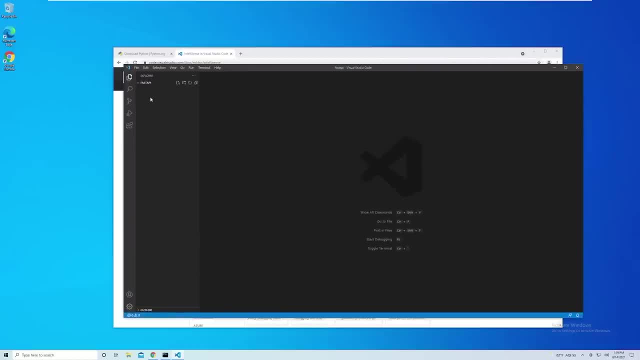 welcome menu. And so now what we have is we've opened up whoops, we've opened up VS code And within VS code, we've opened up our project code. So right now there's no code. that's to be expected, But I want to. I want to do is? I want to create a new file real quick, just. 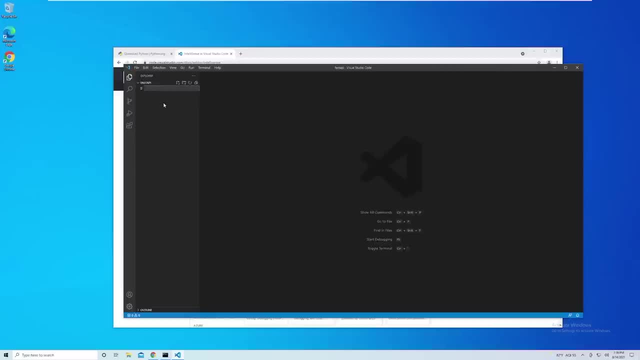 for testing purposes. So I'm just gonna right click, hit new file and I'm going to name it. name main dot py. And so we want to name it dot py, because this is going to be a Python file, And before I hit enter, I want you to focus your eyes right down here. 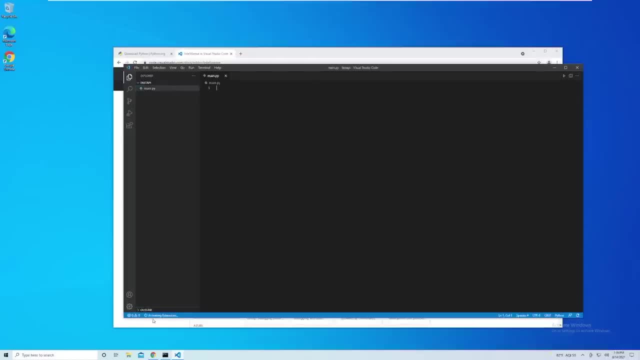 and you'll notice something happens down there. So when I hit Enter you'll see activating extension. So it's activating the Python extension. And what the Python extension is going to do is it's automatically going to select the correct Python interpreter, or it may not be. 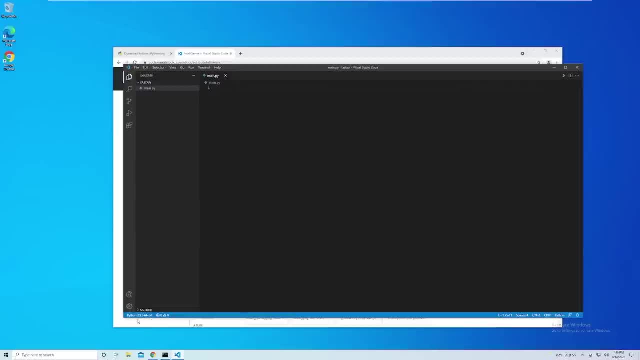 corrected depending on what happens on your machine. For me to automatically detected Python 3.0, dot nine, dot six was installed on this machine, So let's selected that one for me. Keep in mind, if you have multiple versions of Python installed, it may select the wrong interpreter. So what you. 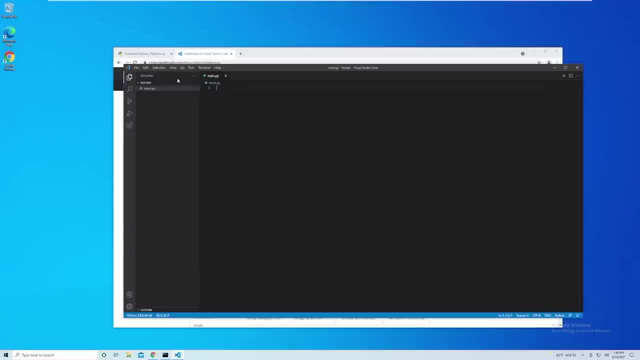 can do is, if you ever want to change the interpreter or specify a specific interpreter, go to view command palette And what I want you to do is search for Python interpreter and then look for Python select interpreter. So right now it's going to highlight where 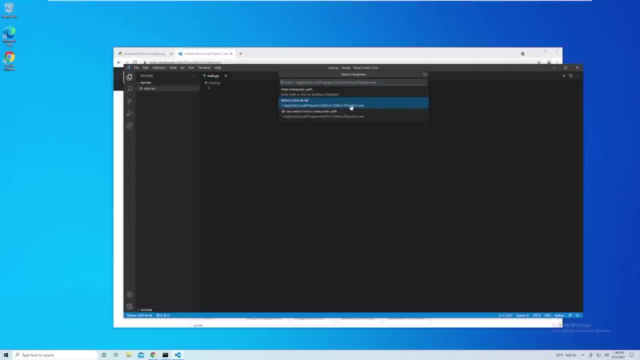 the current Python interpreters, which one selected and what's the executable for it. But if you want to change that, you can select enter interpreter path and then provide the path to the specific version that you want. So you can always change it. But usually it's able to detect. 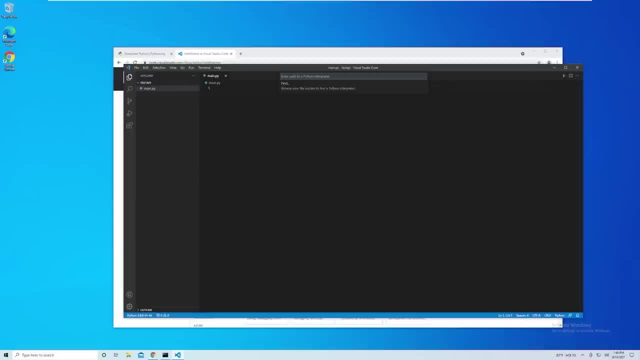 the latest version, So you should be good to go, And so that's all I wanted to do from a setup perspective. There's one more thing that we'll cover later, But we'll get to that in the next section. But right now we've got Python installed and we've got VS code set up And we've got our 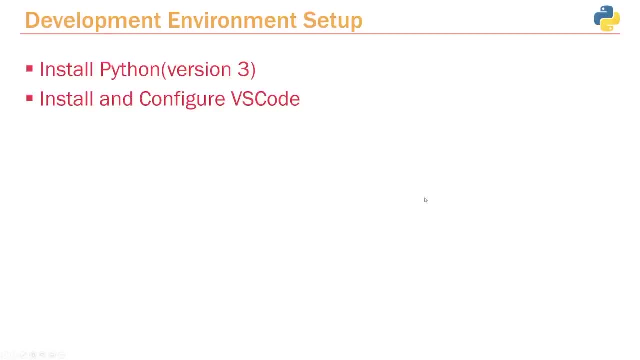 project directory set up, so we should be good to go. So now that we have Python and VS code set up, the next thing that we have to do is set up our virtual environment. Before we do that, we have to actually talk about what our virtual environments. 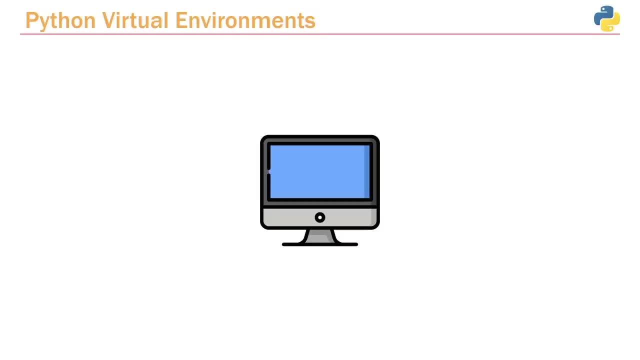 and what problem do they try to address? So let me give you a little bit of an example scenario of the issue that we can run into when working with specific packages within Python on your local machine. So let's say that we created a project and this project is called project one, And what? 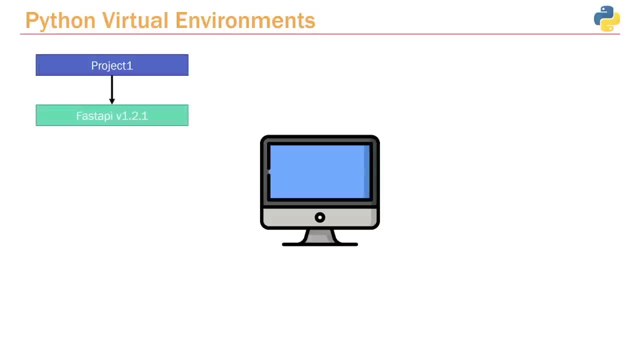 we need to do is we need to install fast API version 1.2.1.. So what do we do? we install version 1.2.1 on our machine so that we can actually use that version. Now let's say later: 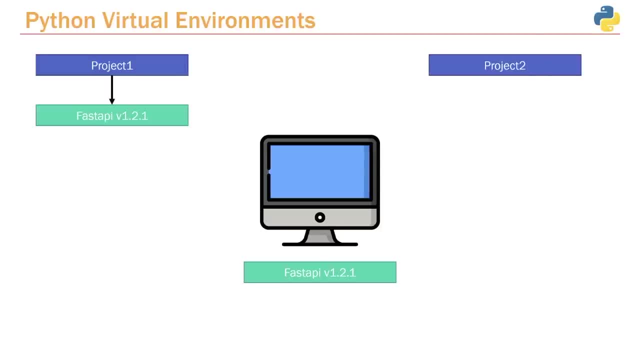 we start a new project called project two And let's say this version requires us to run fast API, version 2.4.3.. Because we want to try out some of the newer features. Well, at this point, if we need to try out a newer version, we have to upgrade fast API to version 2.4.3 on our 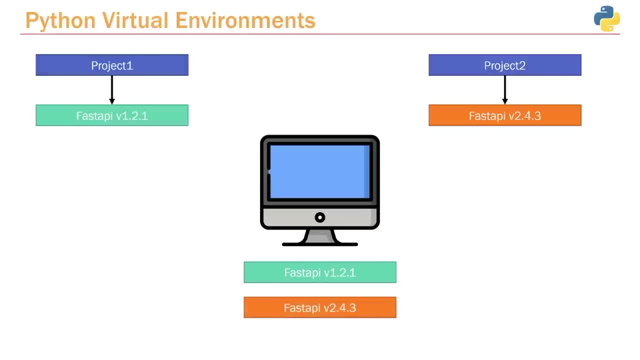 local machine And this may or may not be a problem. it really just depends on if version 2.4.3 is backwards compatible with version 1.2.1.. Because if version 2.4.3 has breaking changes, 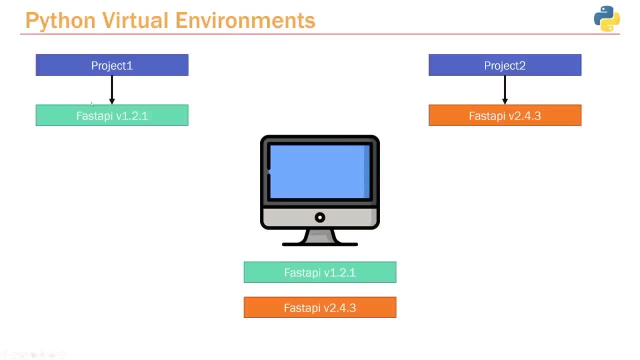 then ultimately that's going to create issues with our project one, because that project expects us to run version 1.2.1.. And so if we can upgrade, well, we're in a little bit of a pickle, because one project needs one version, the other project needs another version. we can have two. 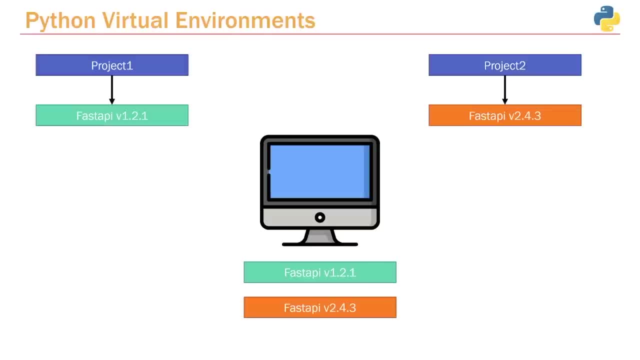 different versions installed on our machine. So what exactly do we do? Well, this is where virtual environments come into play. So, with virtual environments, let's say we want to create a project, So we create project one, And what we do is we create a virtual environment. call it. 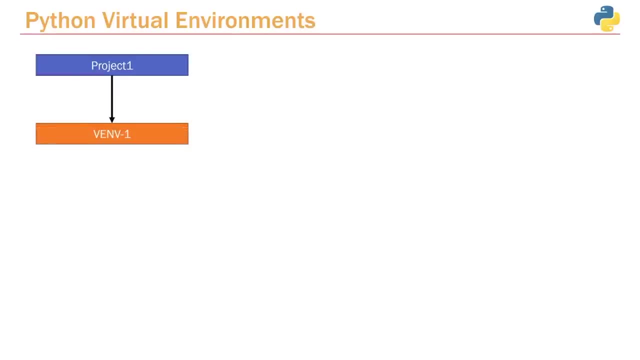 whatever you want, And so this is a isolated environment And this is a virtual environment that will not affect any other environments, And within this environment we can install any Python packages running whatever version we want, and it's completely isolated to this project And 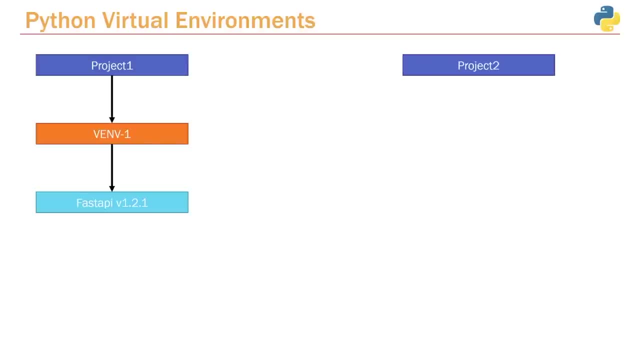 so when we create a second project, what we can do is we can create its very own virtual environment as well. we'll call it virtual environment two, And within this virtual environment we can install any version of any package that we want, So then we can install version 2.4.3.. And so both of these. 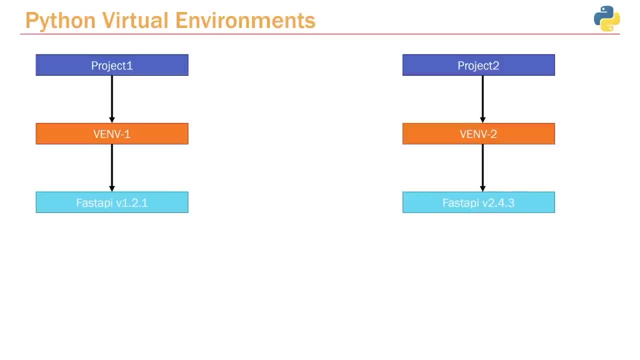 virtual environments are completely separated, completely isolated with one another, And so we can essentially install multiple different versions of a single package for each of our projects, And that way our projects don't end up stepping on the toes of other projects. And so now, 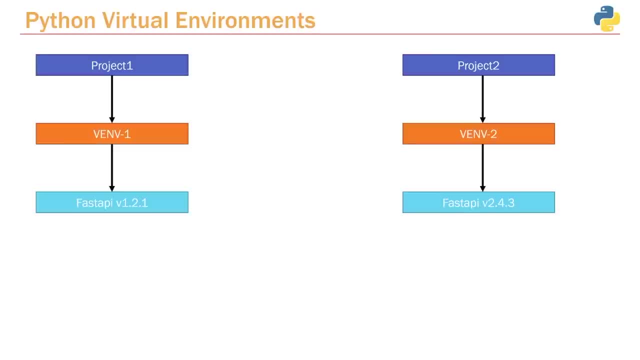 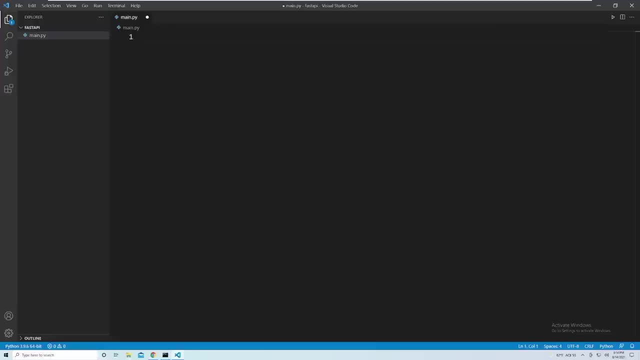 that we have a basic understanding of virtual environments, let's go ahead and figure out how we can actually create our first virtual environment and use it within our project. In this video, I'm going to walk you through setting up a virtual environment on a windows. 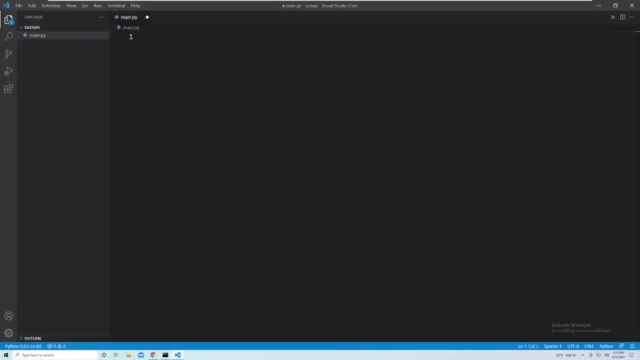 machine. Now, if you already closed out your VS code window, go ahead and open up a new one and make sure you open up the specific directory we created a couple lessons ago. Now what we want to do is we want to select terminal. 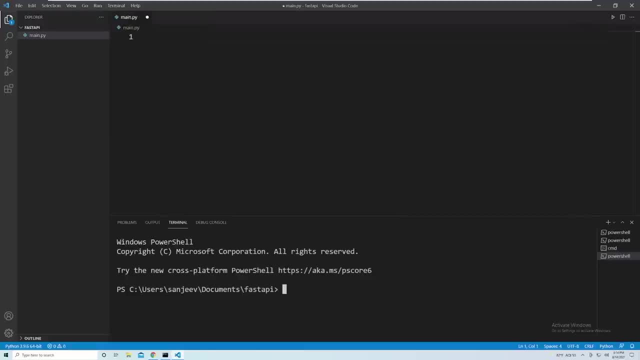 and we want to select new terminal, And this is a awesome feature with VS code. it allows us to have a integrated terminal within our VS code window, And this terminal is fundamentally no different than a regular terminal within Windows. It's just built into VS code so that we don't have to keep. 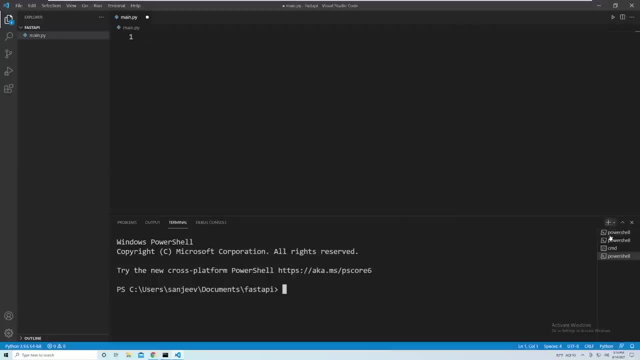 flipping between different windows, And if you actually take a look at this right column, we can have multiple terminals open and we can even use different terminals. So the default one on this machine happens to be PowerShell, But you can also use Command Prompt if that's what you prefer. 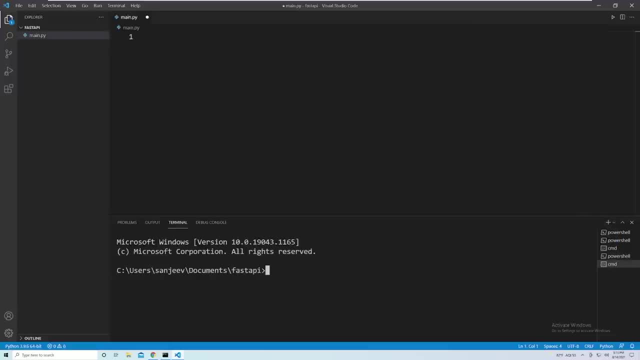 So if you select Command Prompt, it's going to create a new terminal And you can see that this is a traditional command prompt. I'm going to use this one because that's the one I normally use. However, if you're more comfortable with PowerShell, feel free to use that. 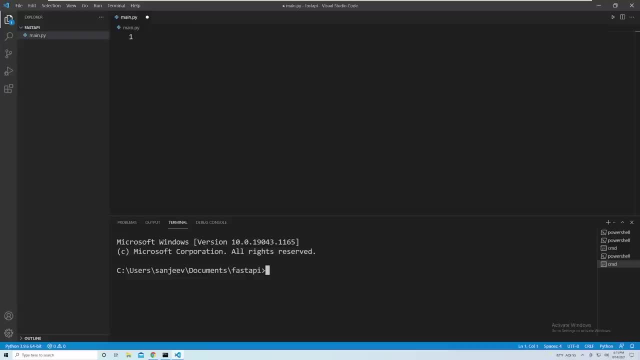 Now the command to actually create a virtual environment within Windows is py dash three dash m, vn v. So that stands for virtual environment, And then you want to give it a name. So give whatever name you want for your virtual environment. You could name it after your project name, or you could just do what I do, which is just call it vn v. 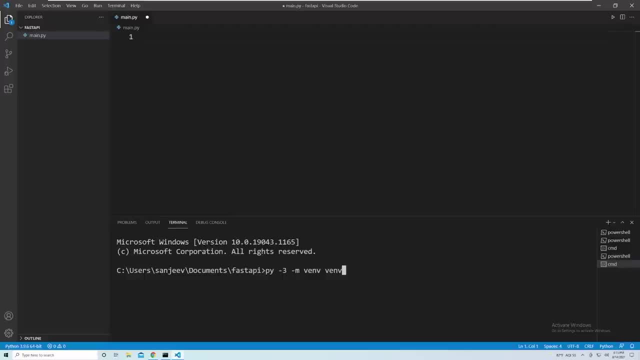 And what I like to do is, for all of my projects, I give it the same exact name, And that's perfectly okay, because this virtual environment is going to be isolated to this project directory, And so, even though this project has a virtual environment named vn v, 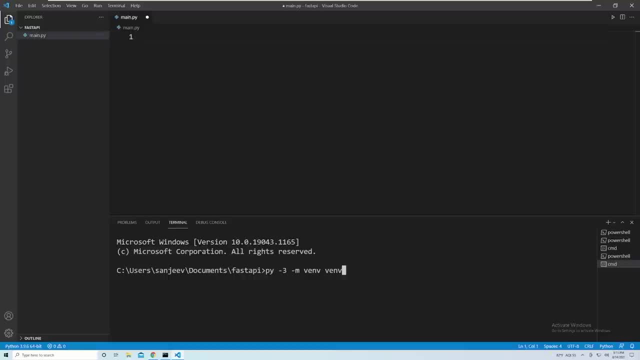 I can create another virtual environment in any other project with the same exact name. they're all going to be isolated to that specific project folder. So go ahead and hit enter And take a look over here. you'll see that a folder was created called v. 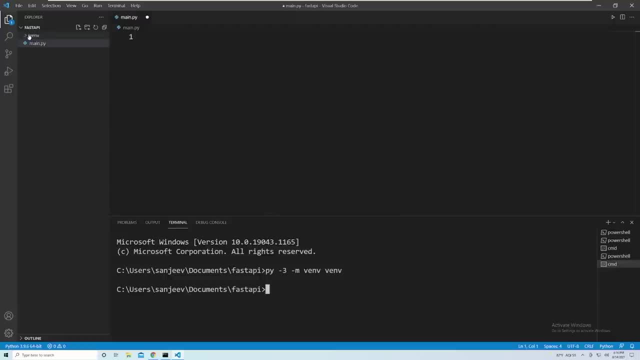 virtual environment, or v? Nv, And that's going to be the name of this folder- is always going to refer to whatever name you gave it. So if I named this cookies, this would open up a new folder called cookies. If you want, you can take a look at what's in here and if you go under scripts specifically, 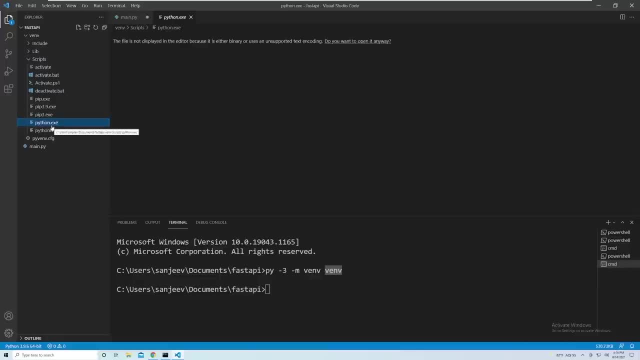 you'll notice that we've got our Python executable, So this is going to act as our new interpreter, And so what we want to do is: right now we are using our global interpreter And we want to change that. we don't want to use it internally, So let's go ahead and hit enter, and we're going to. 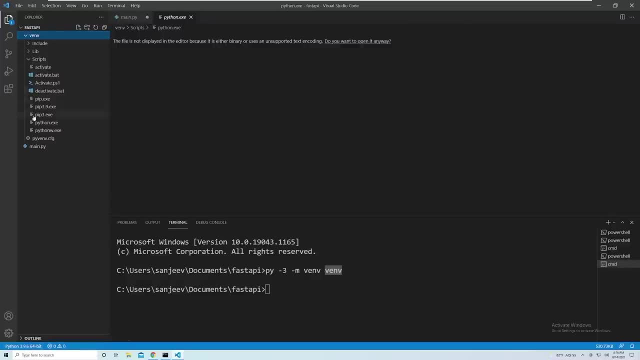 change this, and then we want to say She is called using this product. So we are magic and we're not. that we don't want to use the global one, we want to use the specific one in our virtual environment, And that way we can install packages that are exclusive to just this specific virtual 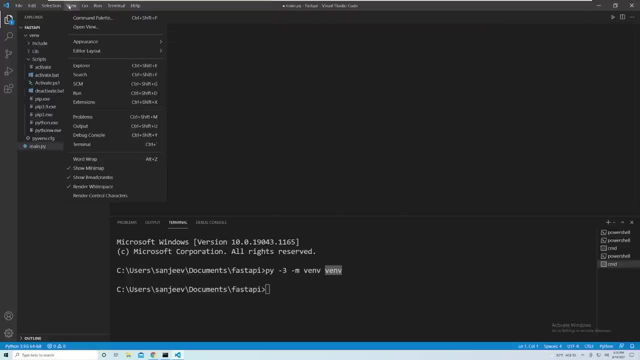 environment, And so, to do that, go ahead and select view once again, And we want to go to command palette and then search for Python select interpreter, as usual, And then you'll see the one we're currently using, but we want to pass in our newest one. So select enter. 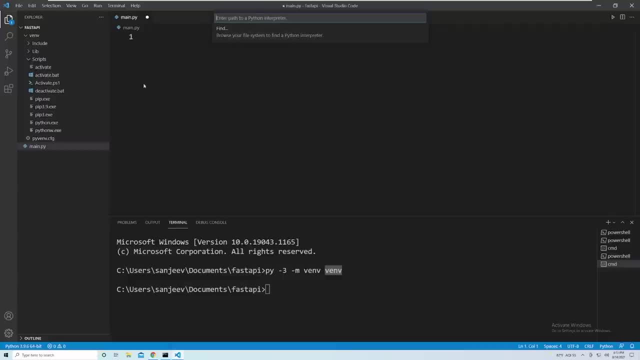 interpreter path. And then we want to give it the path to our interpreter, which is the path from the root of our project directory to this pythonexe file. we're going to say dot, which is our current folder, So this is going to be the fast API folder And then within here, 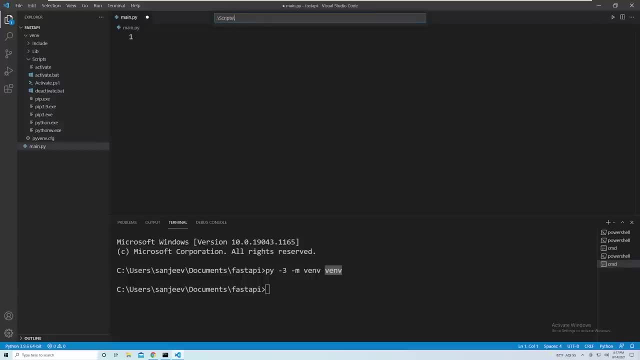 we want to go into scripts And then within scripts, well, sorry, we want to go into the virtual envy folder, then scripts And then pythonexe. go ahead and hit enter And then, if you look down here, you'll see the path to our interpreter. And then we want to. 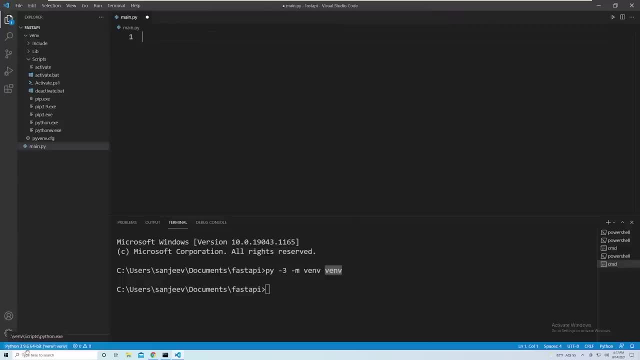 down here, you'll see that this gets updated. So now we're still using three dot nine, dot six, but we're using our virtual environment, And so that's all we need to do, And it should remember this every time we open up our project. However, double check every time you open up, just to make. 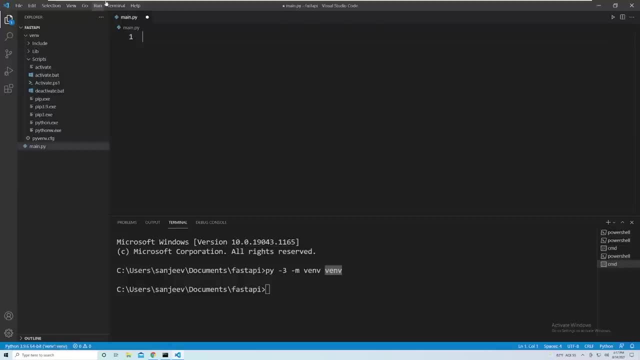 sure you're using that. if it's for some reason moved back to the default one, just do the same process. Now, the second thing that we need to do is we need to make sure our terminal is also using the virtual environment, And so what we want to do to do that is just type in. 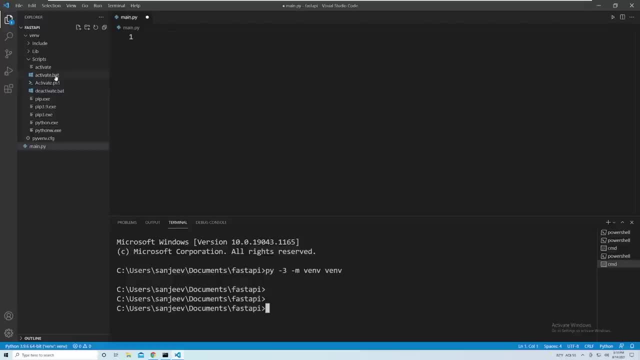 the path to this specific activate dot bat file. This is going to activate that virtual environment within our command line as well. So I'm going to say virtual envy And then we want to pass in our scripts folder and then activate dot bat, Hit enter And then notice what's changed. 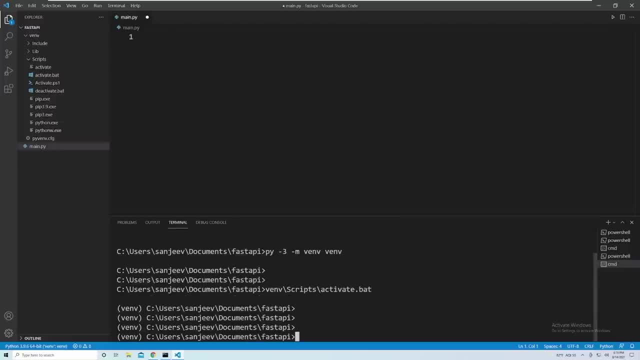 right. So when you're using a virtual environment- right, you're going to see the name of the virtual environment to the side of it. So when you're using a virtual environment, you're going to see the name of the virtual environment, And so always double check whenever you start up VS code and you. 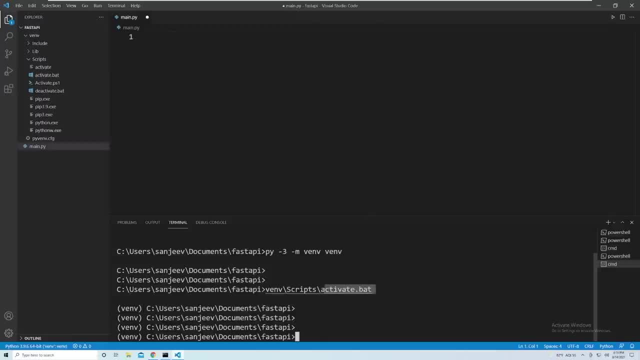 start up your project that this is enabled. If you don't see this, then just run the same exact command And that's going to reactivate the virtual environment. And so at this point we are good to go with our virtual environment and we can start coding out our project. In this video I'm going 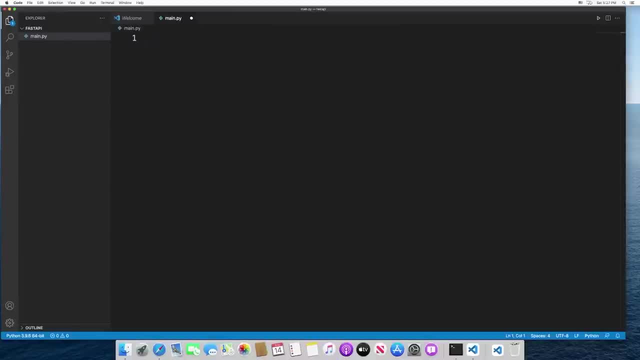 to walk you through setting up a virtual environment on a Mac machine. Now, if you've already closed out your VS code window, go ahead and open it back up, and open up the folder that we created a couple lessons ago. Now, within here, what we want to do is: 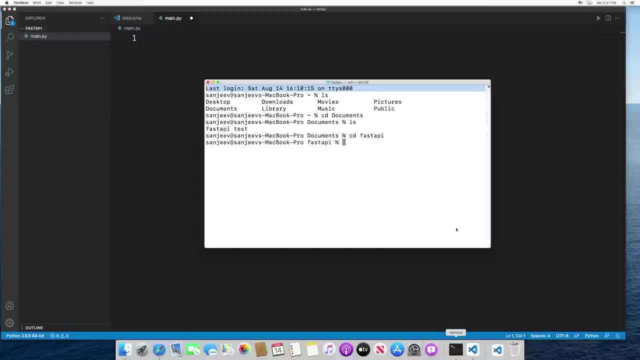 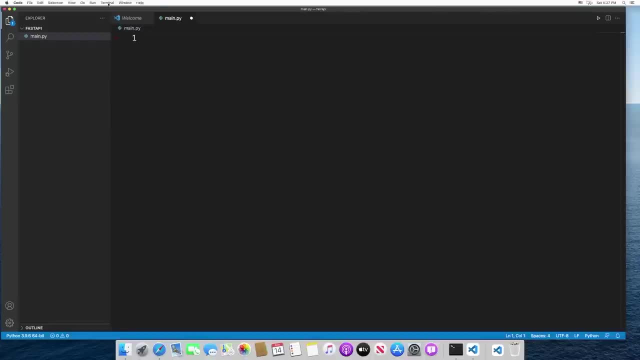 we want to access our terminal. So we can access our terminal just by selecting this And then this is our terminal. However, VS code has a feature where we can access the terminal directly within our VS code window. So if we select terminal and the new terminal, that's going to create a new 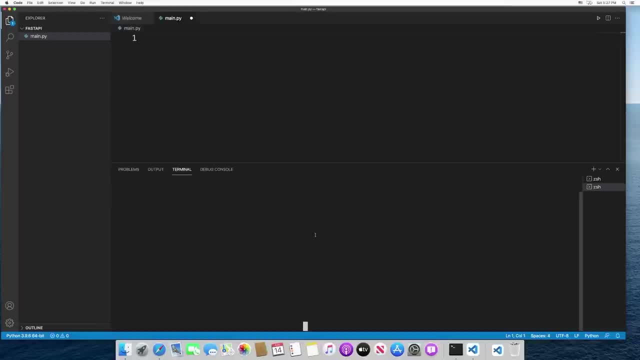 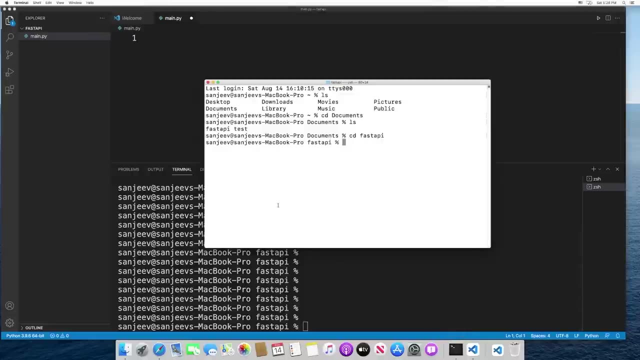 terminal for us, All, right, And so this is fundamentally the same thing As this terminal right here. it's no different, But at least by having a built into VS code, we don't have to keep flipping back and forth between the two, So you can use either one. whichever your preferences, keep in. 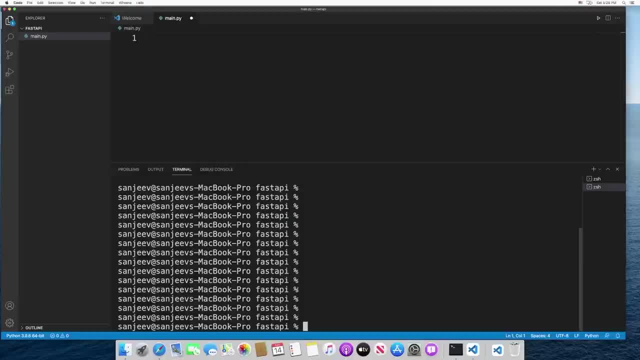 mind that you open up the terminal within VS code, it automatically moves you to the the directory folder of your project, So you don't have to move there yourself. You can use whichever one you want. Now I'm actually using, I'm running Mac on a virtual machine right now, just because I natively use a Windows. 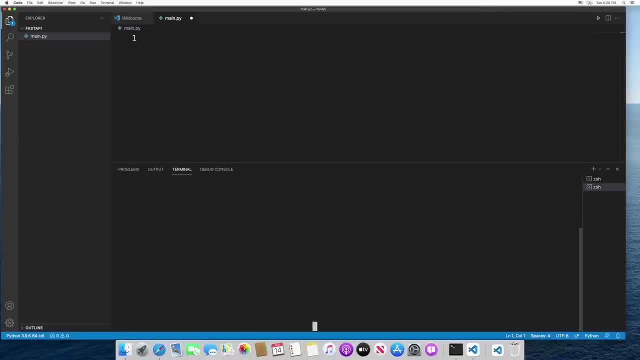 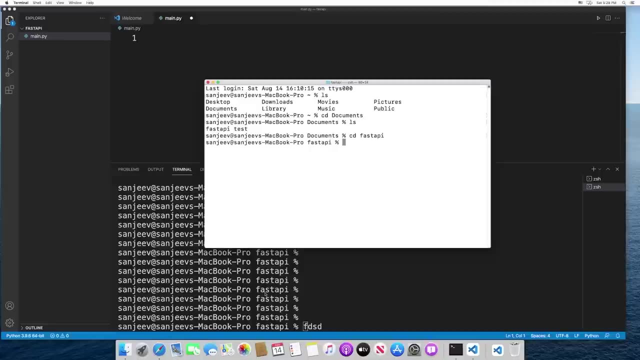 machine. So I don't actually own a Mac. So this is a little bit buggy And if you see me type things you can see advantage. So for demonstration purposes I'm just going to use the regular terminal, But I strongly recommend you use the one built into VS code So you don't have to keep flipping back and 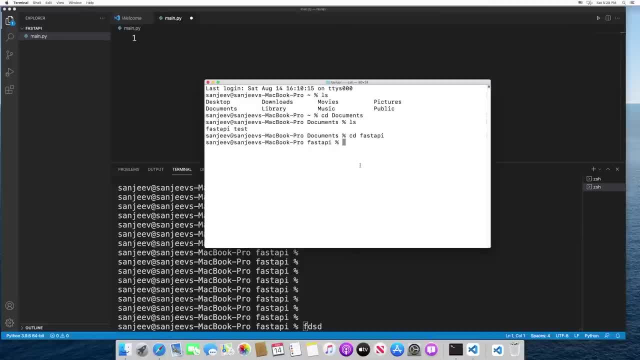 forth Now to actually create a virtual environment. there's one command that we have to run. So you run Python three, dash, m, v, e, n, v for virtual environment, and then you have to give it a name. So what name do you want to give your virtual environment? you can technically give it any name. 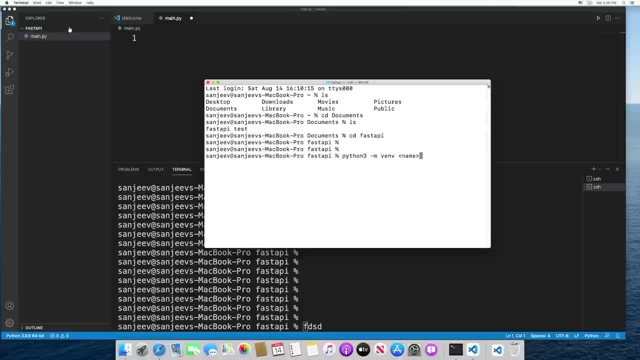 you want. you can name it after your project, you can give it some arbitrary name. what I like to do is I like to name all of my virtual environments v, e, n, v, And so for every project that I create, I just create. 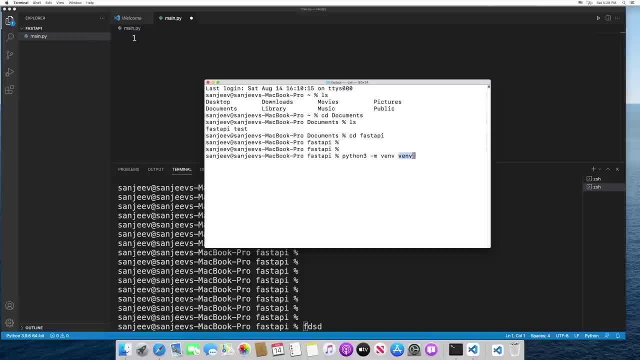 the same exact virtual environment name- v e, n, v- And that's not going to create an issue. it's perfectly okay to name all of your virtual environments the same thing, because it's all going to be exclusive to this specific project folder, So no other projects can access it. So it's okay if they all 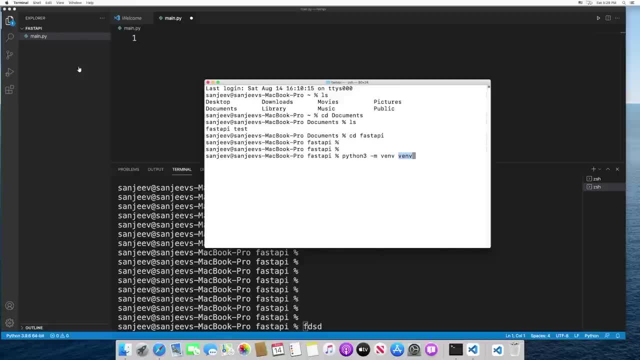 use the same name. it's just easier And so that way you know, if I ever create a get ignore file, I can automatically add v e n v And I can make sure to just use the same exact get ignore template across all of my Python projects. So I'm going to use v e n v And I want to make sure that you pay. 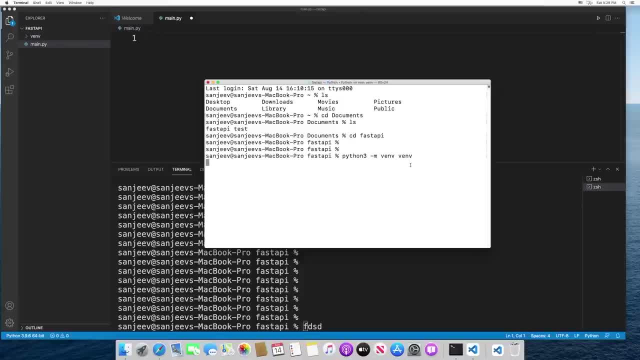 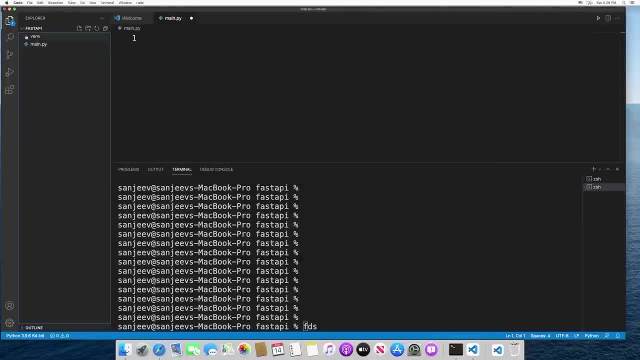 attention right here, because after I've run this command, take a look at what happens. it creates a folder called v e n v And that's based off the name of the virtual environment. If we take a look at our virtual environment, you can see a couple of different files. you can see the, the Python file. 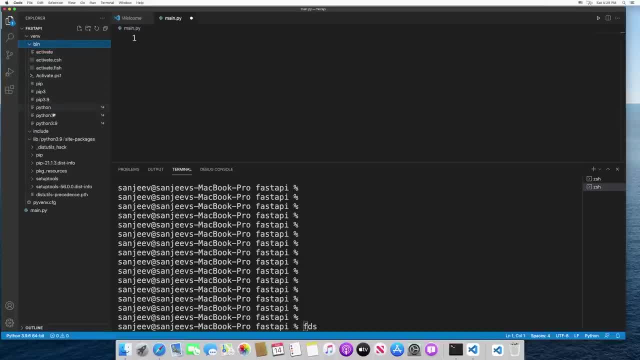 as well. So if you go under bin, this is going to be the new Python file, or the Python three file that we're going to use for our interpreter. So down here at the bottom, you'll see that we are still using the global interpreter. we no longer want to use the global one, we want to use the one. 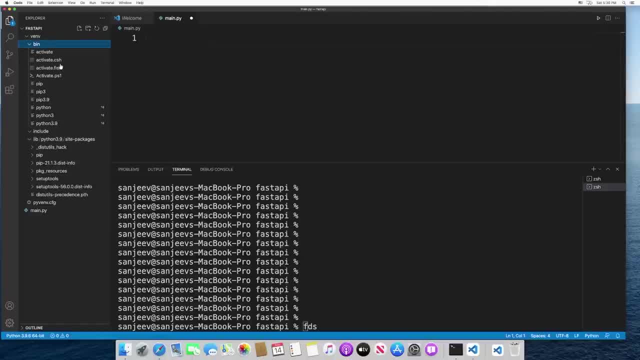 in our virtual environment. That way we don't, you know, cause any issues with other projects. we want to use the virtual environment So to do that. what we want to do is we want to select a view command palette And then we want to do the Python select interpreter again. So we'll select that Right, And 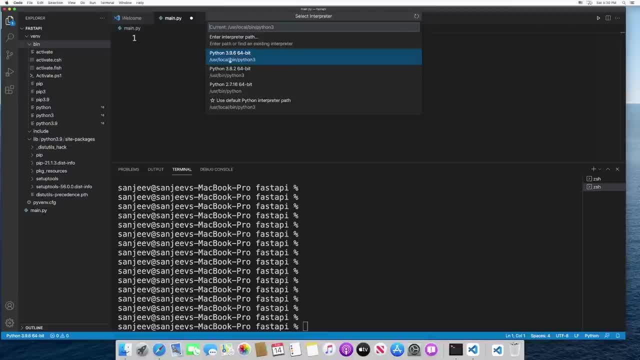 so right now it shows us that we are using the global one. However, we're going to pass in the path to our specific interpreter within our virtual environment, So we'll select enter interpreter path And then we'll say dot for current directory, And so that's going to mean the current fast API. 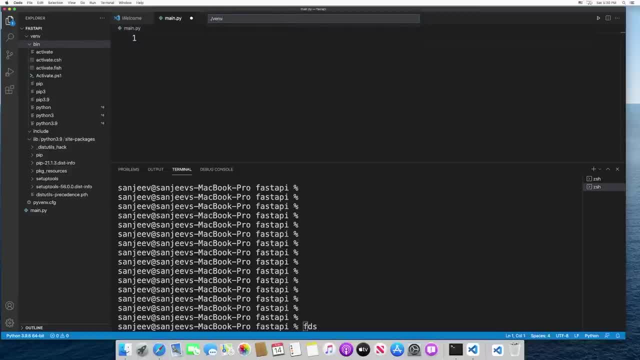 directory, then within there we want to go into the virtual environment folder, And then within there we want to go into bin And then just say Python, And so we'll hit enter and then take a look at what happens down here, Right? you notice that the 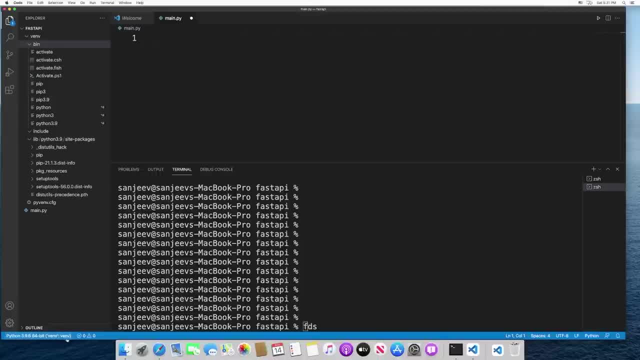 version still says 3.9 dot six, but our interpreter is actually pointing to our local virtual environment now, because we changed the interpreter to use this specific Python file right here, And so this is what's going to allow us to install our own specific fast API. 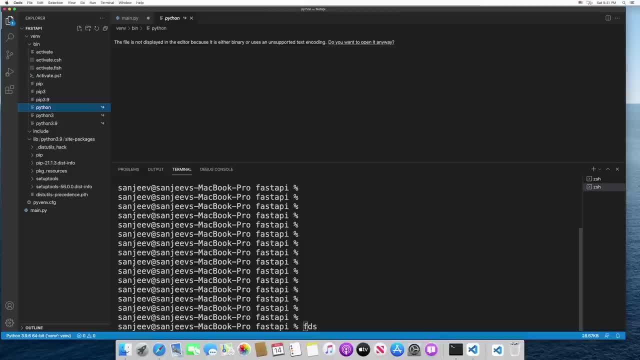 version as well as any other version of any package that we want, So it doesn't actually install it globally on our machine. Now we're almost done. But there's one other thing to note: if you look at our terminal, our terminal isn't using our virtual environment. So if we run pip, install any package. 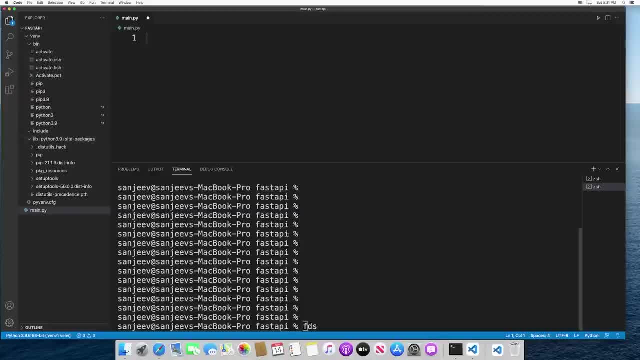 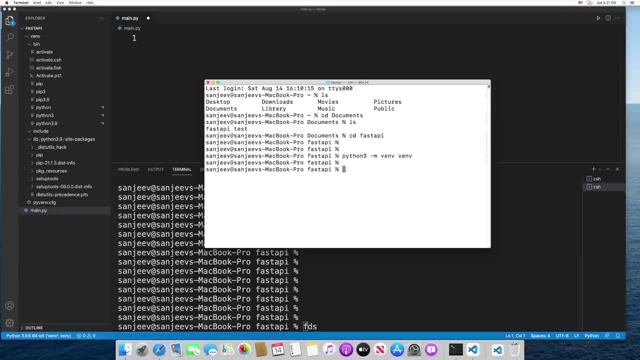 it's not going to install it for a specific virtual environment, it's going to install globally. So we have to enable the virtual environment for the command line as well, And to do that all you have to do is type in source, And then we want to pass in the path to this specific activate. 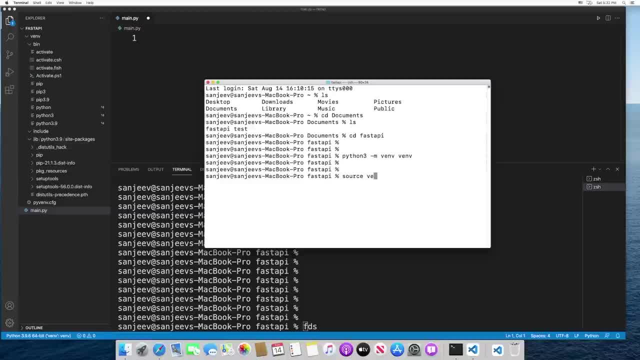 file right here within bin. So we do venv slash, bin slash, activate, hit enter And then notice how our command line changes. Now it's prepended by the name of our virtual environment, So since we named it venv, you can see that it shows it right before the terminal, And so that's all you have to do. our 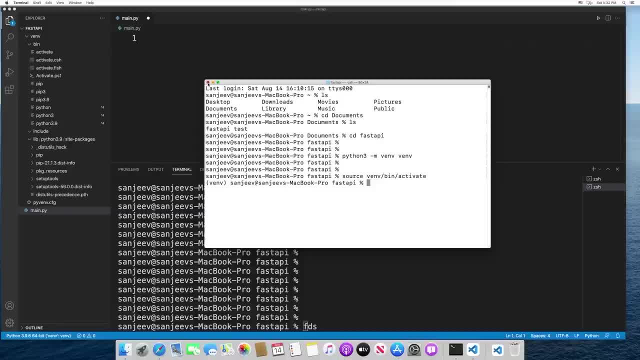 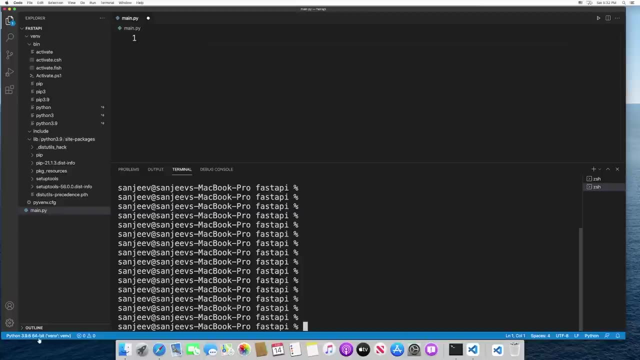 virtual environment is set up. Keep in mind: if you close out your terminal and then reopen it, you'll notice that your virtual environment is gone. So you have to run that same exact command every time you open up your terminal to ensure that you are in your virtual environment, And anytime you close out VS code, make sure that. 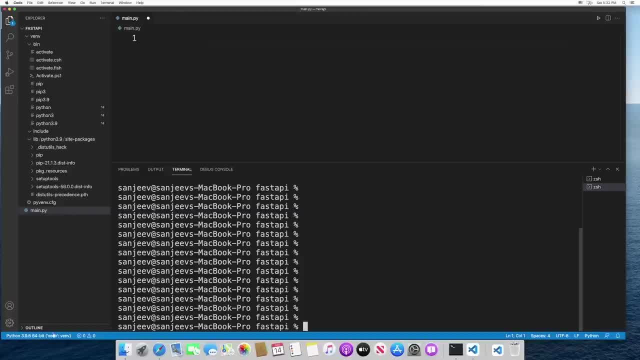 when you reopen your project, it still points to the virtual environment. If, for some reason, it changes, then just go back to that command palette by going to view command palette and then selecting the interpreter that you specifically want, And that's all we have to do, guys. So our virtual environment set up, And so at this point we can go ahead and get started on coding out our project. 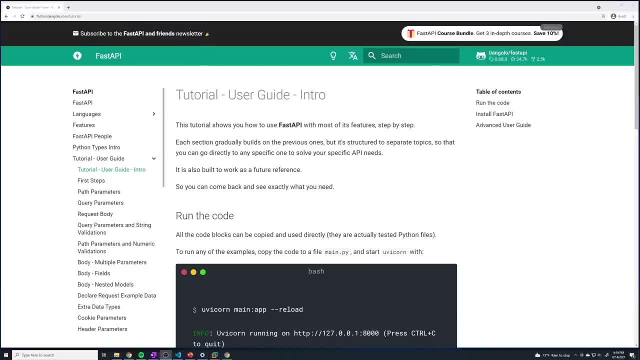 So, now that we got our environment set up, it's time to get started coding out our project, And what I want you guys to do is, first of all, go to the FastAPI documentation. this is really important. What I want you guys to do is really get a solid understanding of how the documentation works. So pull up the 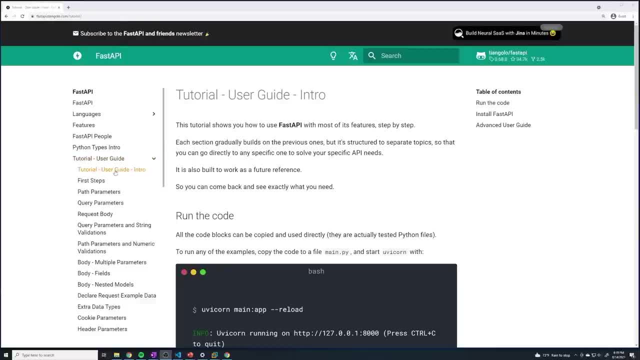 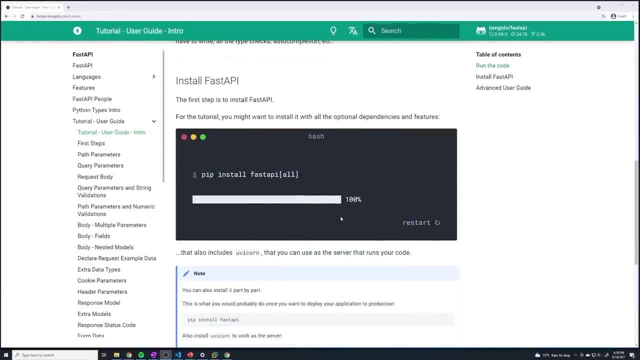 FastAPI website and then head on over to the tutorial section and then select the intro part. So this is going to walk us through setting up our project, And what we will need to do is, first of all, we need to install the FastAPI package, And so what we can do is we can either do PIP, 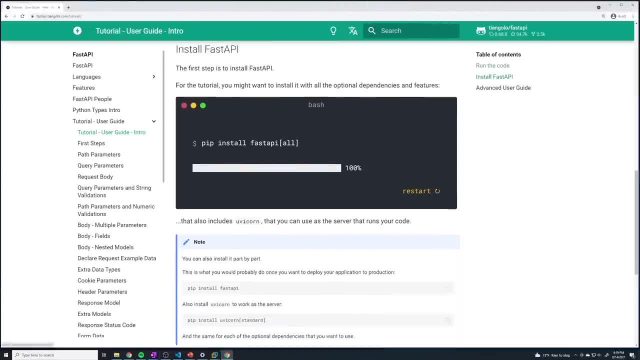 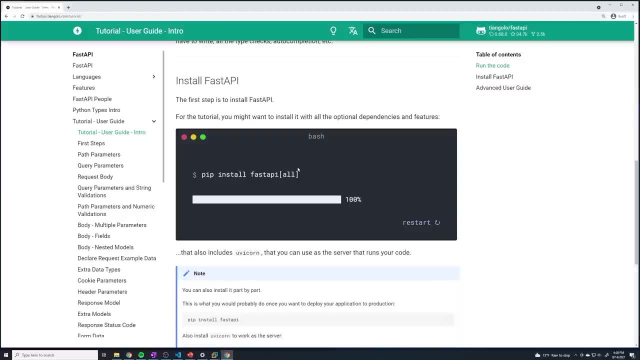 install FastAPI. Or we can do PIP, install FastAPI, Or when we do that, PIP install FastAPI. all it's going to install all of the optional dependencies as well, which we may or may not need, depending on what features we want. we're going to go ahead and use the All option because we're going to use a Hollywood. 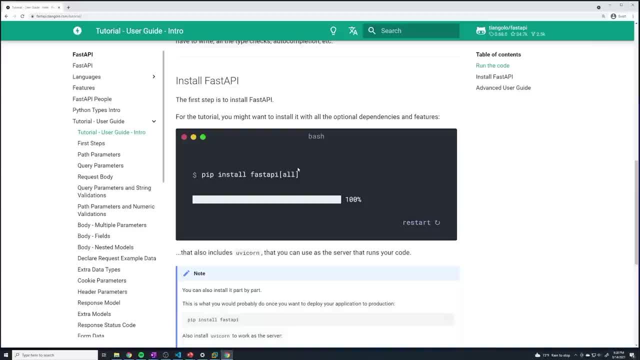 We're going to go ahead and use the All option, because we're going to use a lot of them and there's no point in having to go one by one and install project, And what we would need to do is, first of all, we need to install the FastAPI package, which will stop making any changes on the system, And so that's what we need it to do. 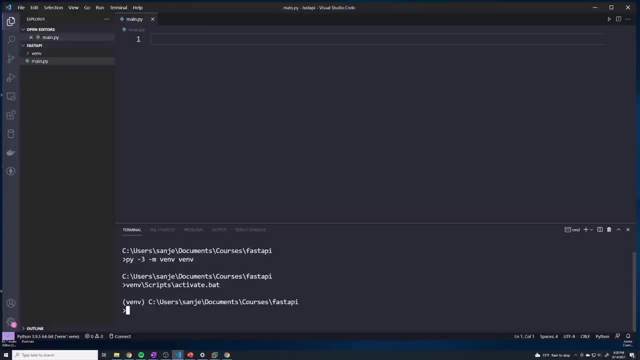 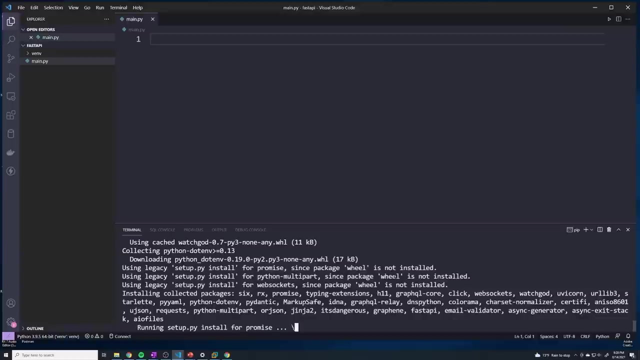 one by one and install them. So that's what we're going to do. So here in our command line, and make sure that we are in our virtual environment And then just type in pip, install fast API, And then we'll pass in all and we'll let that run. Now it's moving fairly fast. 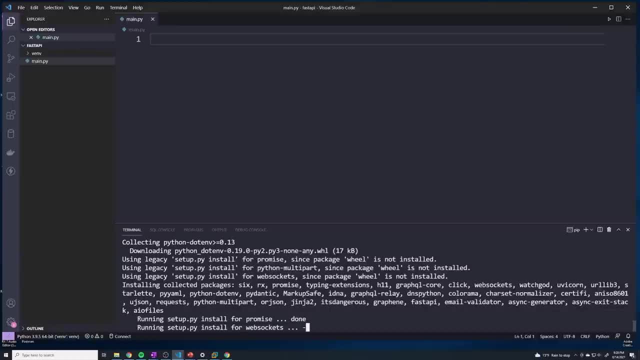 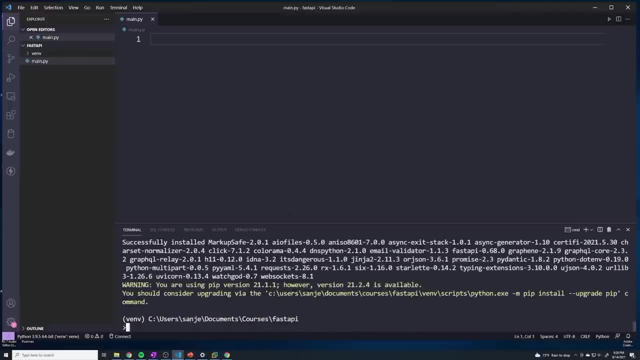 But if you kind of scroll through the history you'll notice a lot of packages and a lot of dependencies that are getting installed. So we'll take a look at those once it's done, just to see what are the different dependencies that were installed. And so now that that's- 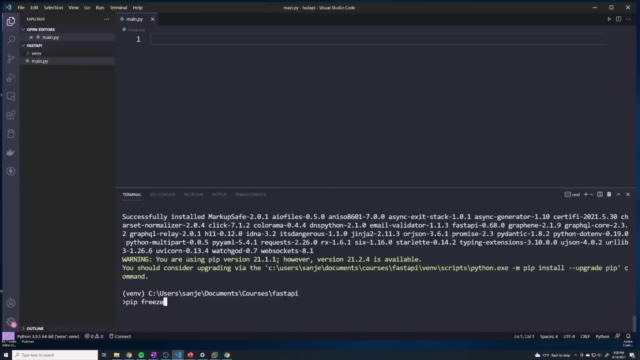 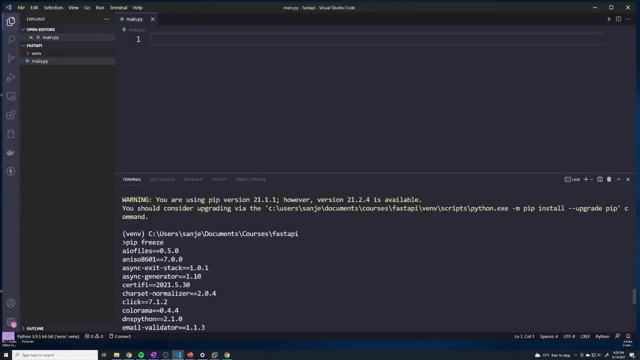 done. if we type in pip freeze, this is going to show all of the packages that were installed. So it's not going to be just fast API. it's going to include a lot of the optional dependencies as well. So if we take a look, you can see that we've got Graph QL installed if we want. 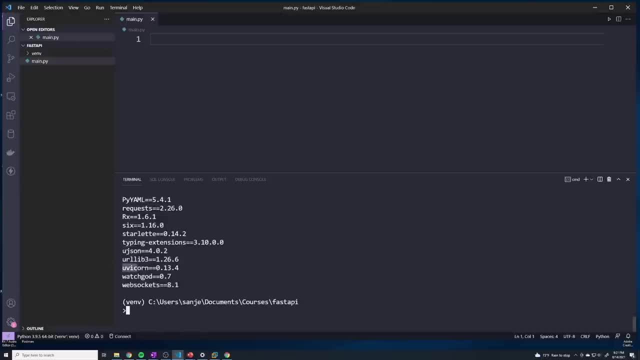 to use any Graph QL. we have bcrypt UV coin. that's going to be like our web server, web sockets. we want to work with WebSocket, So it already comes bundled with a lot of things that we're going to use, And I just wanted to show you a couple of things that we're going to use. So we're going to 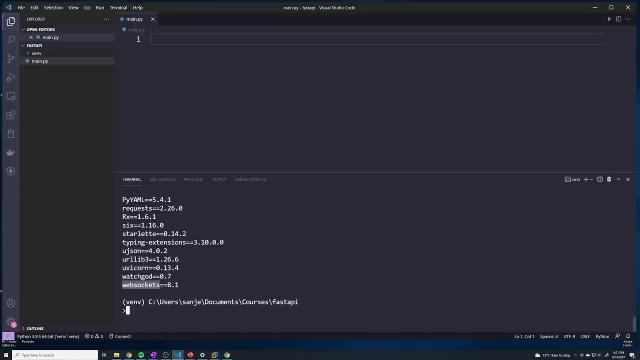 make sure that you guys understood what's happening when we pass in that that all flag. And, if you want to, if you open up your virtual environment folder and you go under lib, you'll see all of the the code associated with those packages that we installed. So 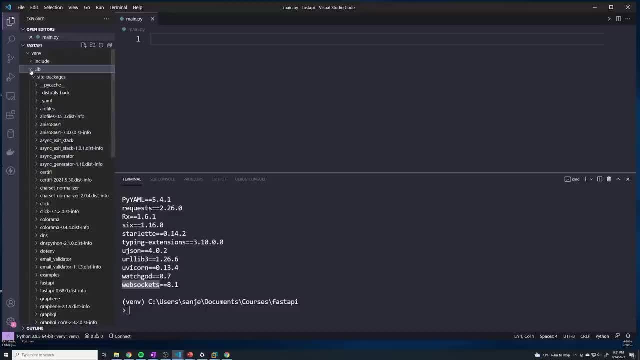 that's where all of them are going to reside. they're all going to reside within the lib folder, Alright. so now that we've got fast API installed, the first thing that we have to do is we have to import fast API. And to import fast API, we just say from fast API. 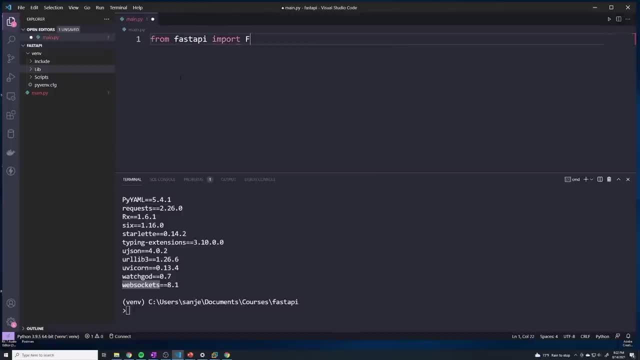 which is the name of the library. We import fast API. Alright, so if we've now successfully imported fast API, let's create an instance of fast API. So we'll say app equals fast API And then we'll call that function. Keep in mind, you can name this anything you want, But if you take a look, 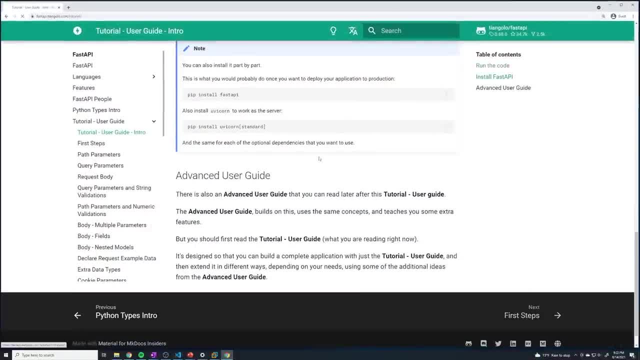 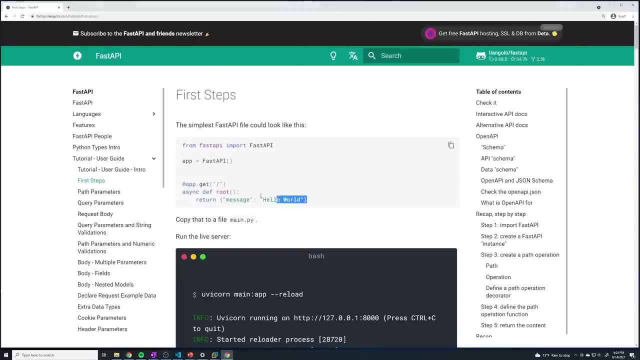 at the documentation and just follow along, you can see that it's going to name an app. So I think it's best if we just kind of follow along with that convention. then what we're going to do is we're going to just copy this code right here. So this is going to be a 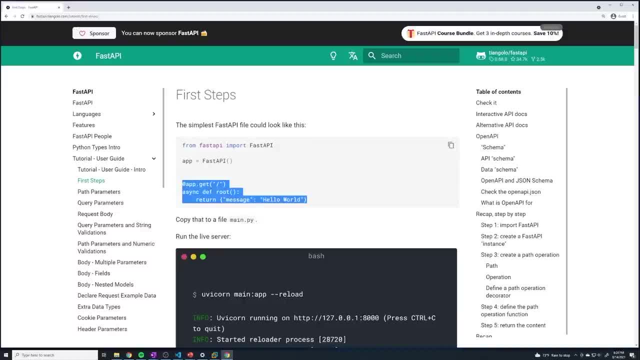 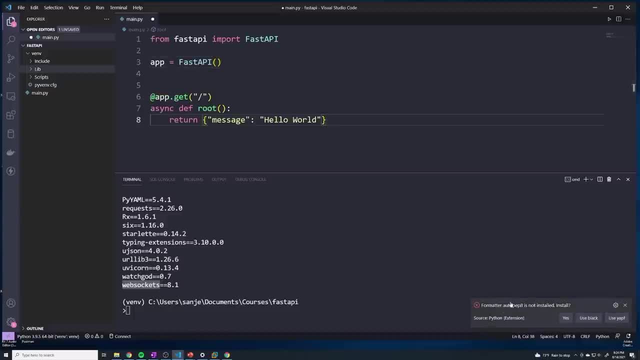 path. So this is going to be what's referred to as a path operation, And we'll go over what that means in a bit And we'll just paste this here. I want you to save your code. you'll see if you get this warning or this message saying format or auto: pep eight is not installed. 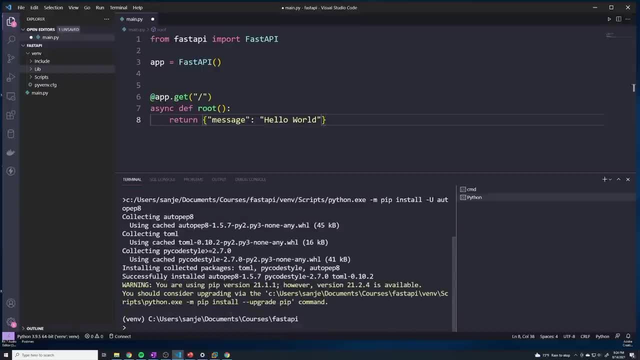 go ahead and hit Yes, And so this is nice because it will automatically format our code. So if we ever put too many spaces or things like that, you'll see that as soon as you save it, it's going to snap into place and make everything look nice and pretty. So let's. 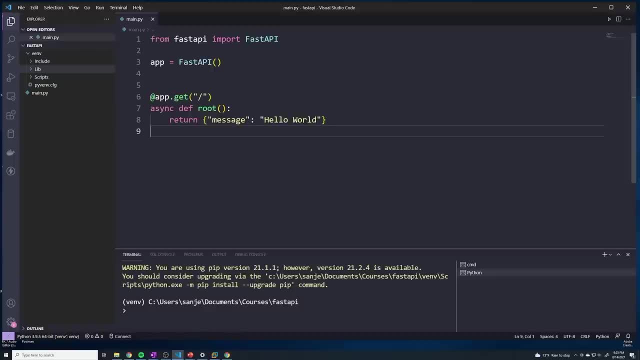 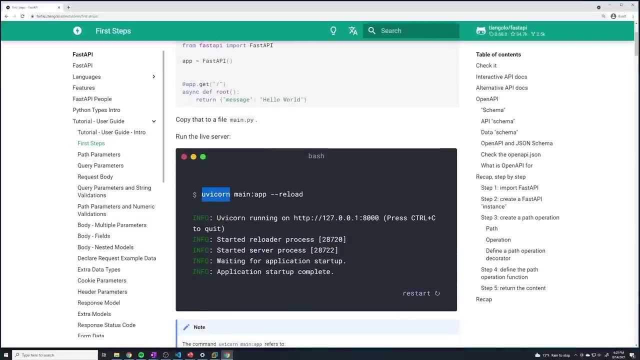 save this. And so, once we've got our code, let's actually start our web server up. So how do we actually start our web server? Well, once again let's go to our documentation. So we're going to make use of the UV corn library. So, because we installed a fast API, 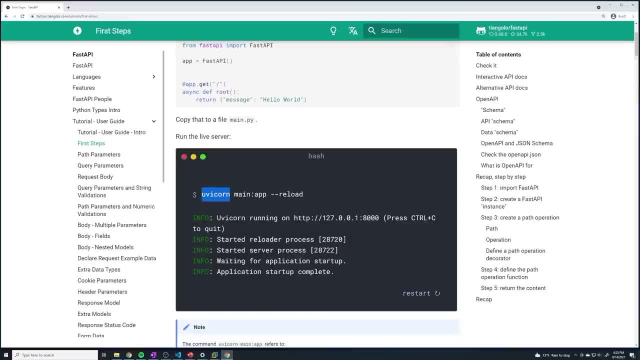 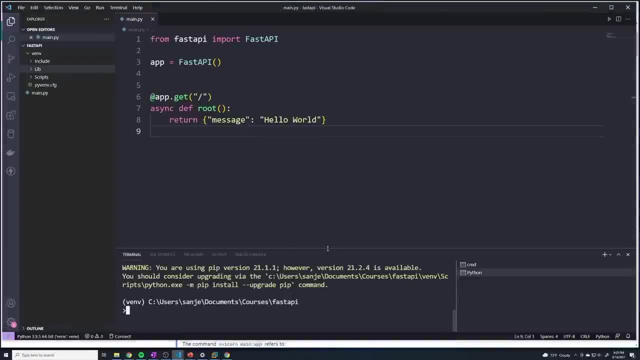 with the all flag, it automatically installed UV corn. if you didn't use the all flag, then you'll have to do pip, install UV corn as well. But we already got it installed, And so let's go back here And let's run our API So we do UV corn. then what we have to do is we: 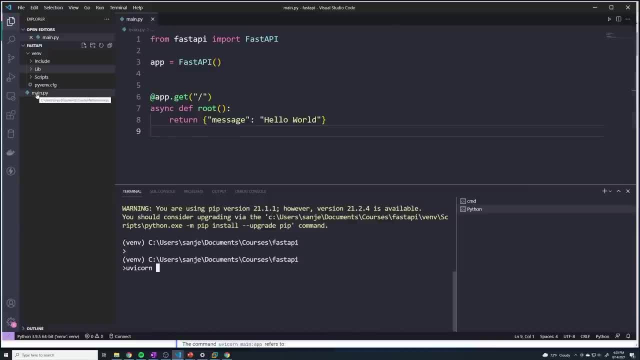 have to reference the name of our file. So this is their entry point into our file. So this is our application, which is our main file. So here we're going to say main, keep in mind, if this file was named anything else, you don't have to name it. main you can name. 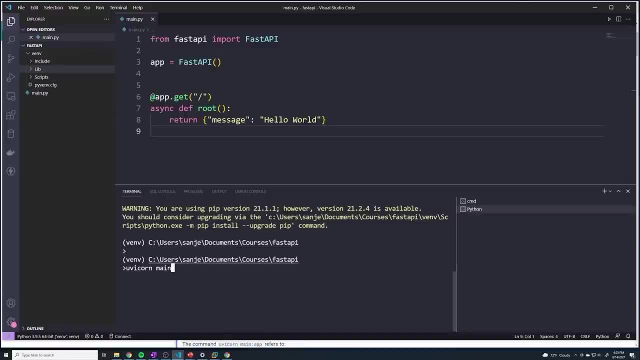 it anything else. you would just want to pass the name of whatever the file name is. then you do colon, then you pass in the name of your fast API instance. So we named it app, And so we'll do app, And then we'll start that Right. And so this is saying that we. 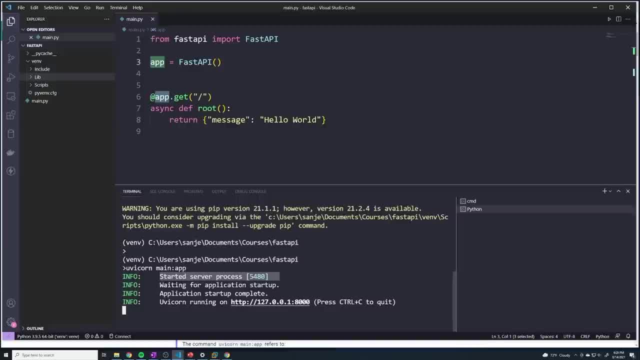 started our server Perfect And we could see the URL that our servers running on. So it's going to say HTTP colon slash, slash 127, dot zero, dot zero to one. So if you guys do don't know what that address is, that means it's this machine. So whatever IP address. 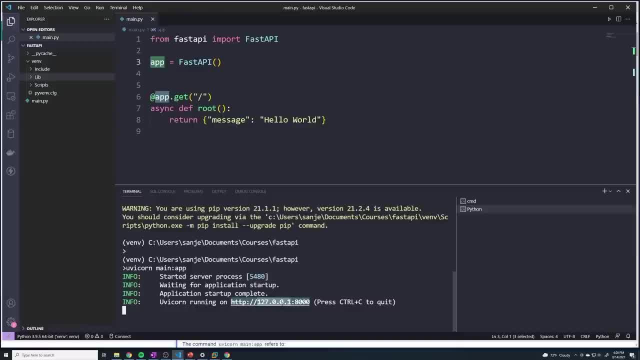 this machine runs on. that's what this is going to be, So it's just saying a we want to refer to the localhost, And it's going to run on port 8000.. So if you want to, you could just copy this URL, go to your web browser, paste it in here and then see what happens. 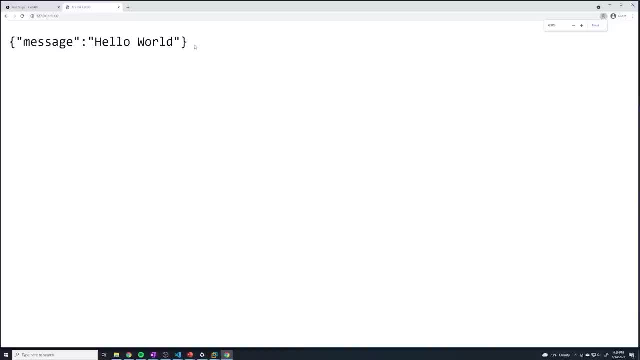 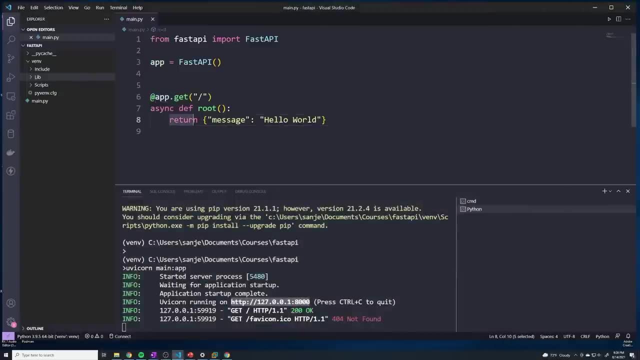 And then look at this, I'm going to zoom in for you. It says: message: Hello world. And that's coming from our code, Right, And that's coming from this return statement. So we're going to use this return statement right here So that. so this kind of verifies that. 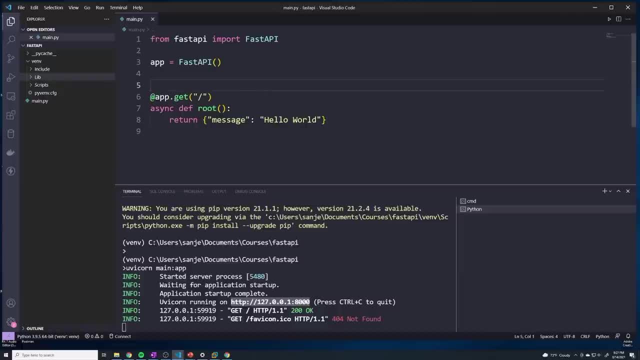 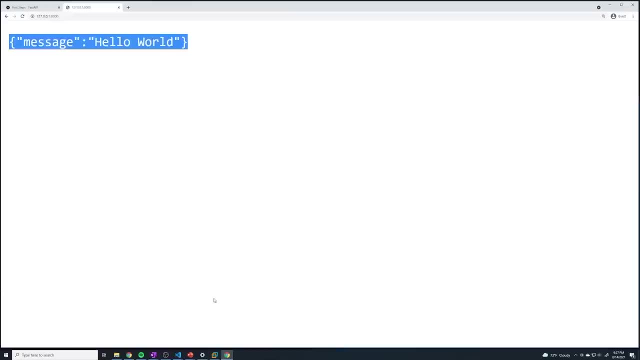 everything worked perfectly Alright. so now that we've got everything up and running and working and you can see that when we go to our website, we can see that we are properly getting back our message, Let's pause this video And in the next video we'll take a. 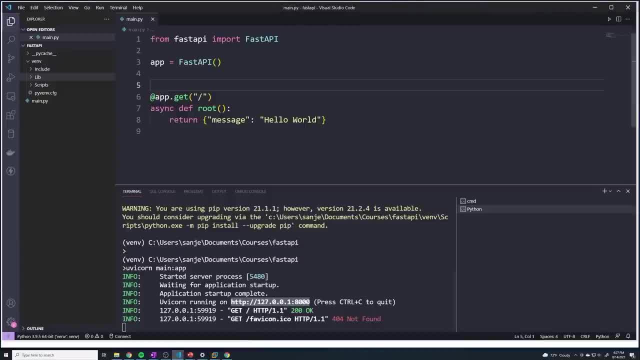 look at exactly what each line of this code actually means. Alright, guys, so let's take a look at the code that we added and actually dissect what each line means. So we've got these three lines of code And if you take a look at the 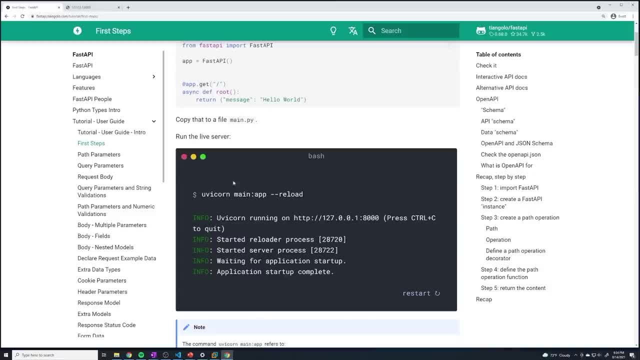 fast API dot com, you'll see that we've added a line of code. And if you take a look at the fast API dot com, you'll see that we've added a line of code And if you take a look at the documentation that we were on, it's going to define those three lines of code as a path. 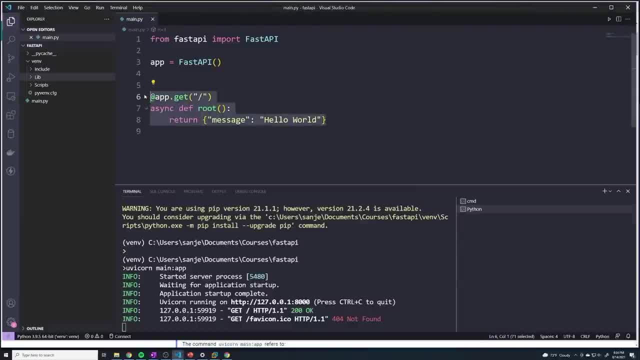 operation. So that's the terminology is using. it refers to this as a path operation. Now, the name itself doesn't really matter. You'll see that in other web frameworks, especially in other languages, sometimes they refer to this as a route, But they within the documentation. 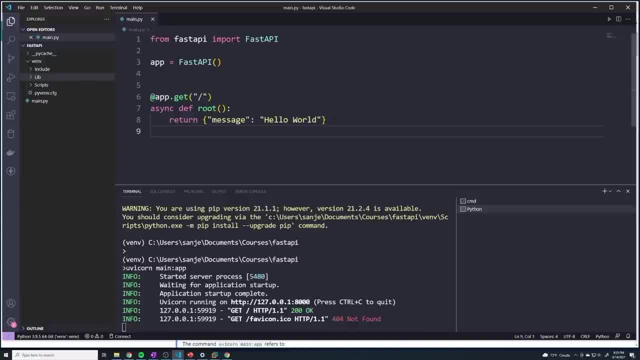 for fast API refer to as a path operation. So you'll see me flip between those two terms, but they fundamentally mean the same thing. So let's actually take a look at this specific path operation And we can really see that it's made up of two components. So we have 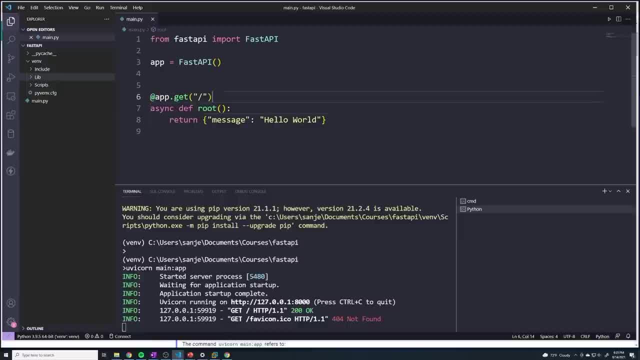 two components. The first component is going to be the function And the second thing is going to be the decorator. So we'll come back to the decorator in a bit. Let's take a look at this function. So this function is fundamentally no different than any other Python function. 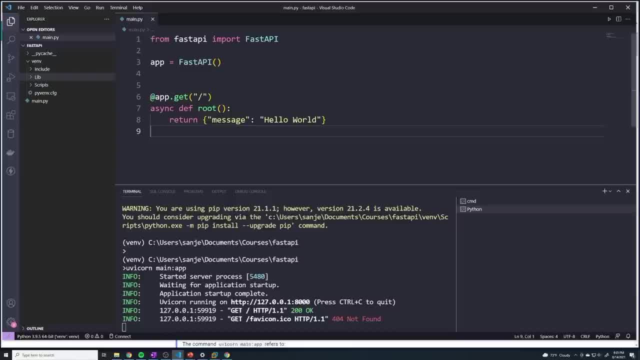 it's a plain old function. you'll see that there's this async keyword. technically this is optional. This keywords only needed if you're going to be performing some sort of asynchronous tasks, So something that takes a certain amount of time, So things like. 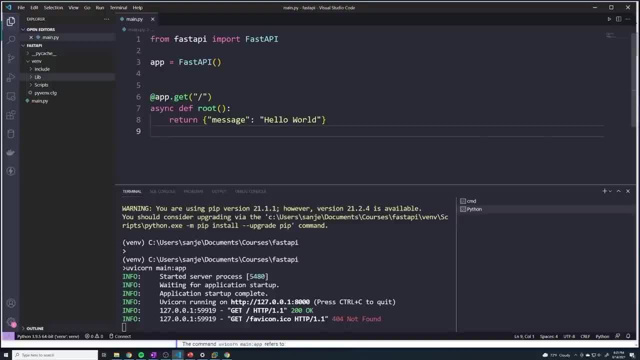 you know, making an API call, things like talking to the database, if you want to do that asynchronously, you do have to pass in the asynchronous Async keyword. but we're not doing that right now. So what we can do is we can actually. 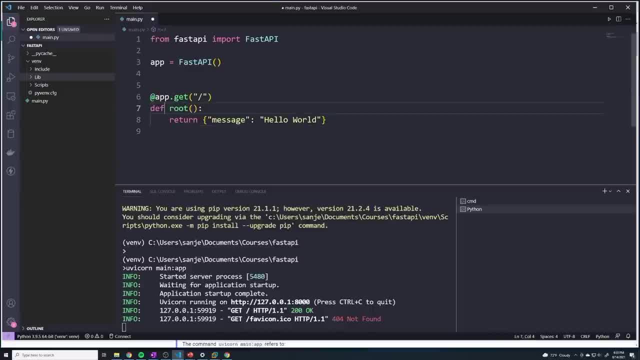 just remove that. So I'm going to delete that and just remove that. And so now it's just a regular function And you'll see that the code behaves exactly the same. So we have a function, we give the function a name, So the documentation just shows an arbitrary. 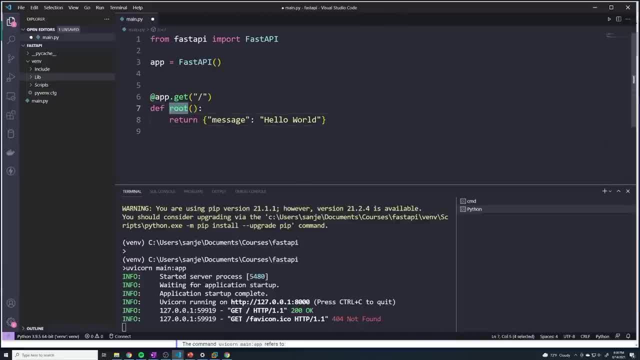 name of route. Keep in mind, the name itself doesn't matter. So if I wanted to name this, you know, get user, then that's going to be fine. it's not going to change anything. It's an arbitrary name. However, I do recommend you name your functions. 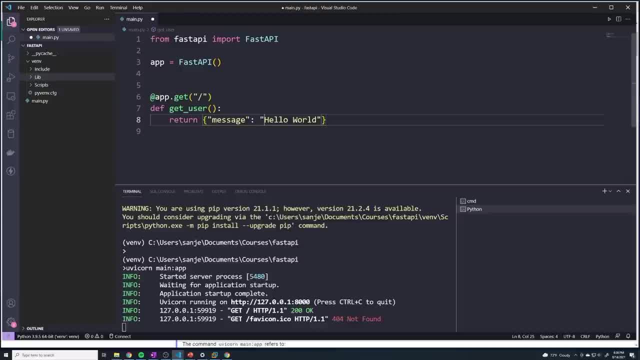 Your path operation functions to be as descriptive as possible. So if you're trying to log in a user, then maybe you should call this login user or just log in, so that it's as descriptive as possible. But keep in mind, the name that we put here does not matter, So I'll change. 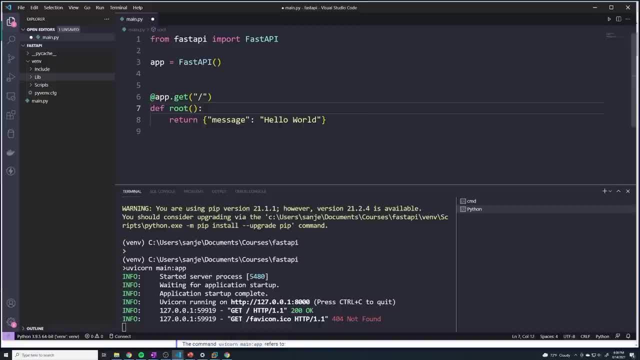 this back to root for now And then we have. so then within this function you can perform any kind of logic. So if this function is meant to log in a user, it's going to have all the code for logging in a user, whatever that may be. So maybe you know. checking the: 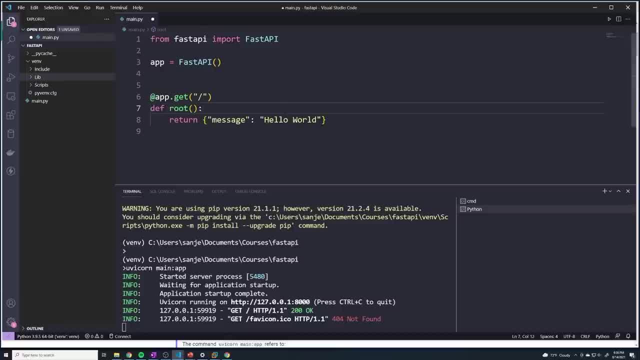 passwords in a database to make sure that they match and to make sure that the credentials are properly accurate, And then after that, you know, just like any other function, we can return something. So whatever we return here is going to be the data that gets sent. 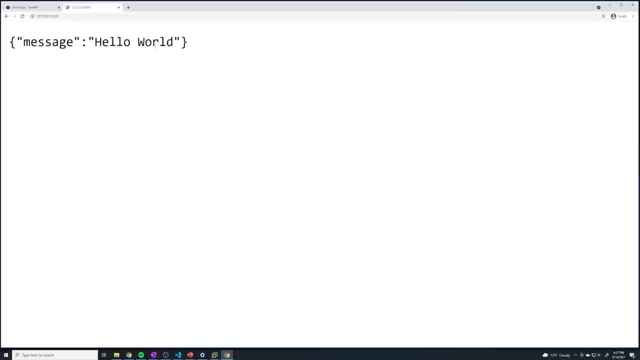 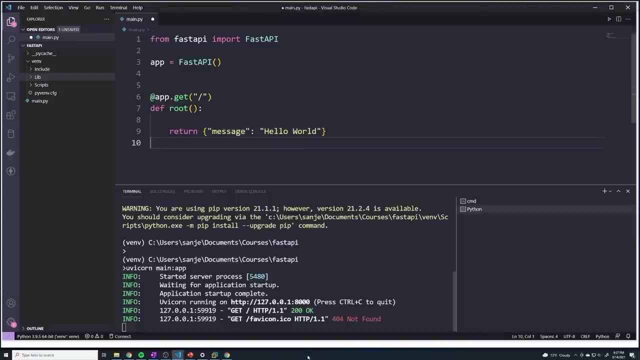 back to the user. So if we go back to the website, go to our web server, particularly this message: Hello world, that's exactly what we sent, And if we change this to be whatever we want, it's going to get returned back in the same way. So here we're just. 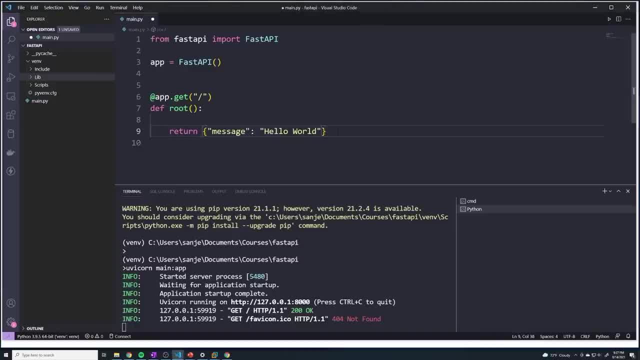 returning a Python dictionary, I guess- And what happens is fast. API will automatically convert this to JSON, which is the main universal language of API- Right, We all talk to. we use JSON to send data back and forth between an API, So it converts this JSON and it sends it back to the user, And that's why we see. 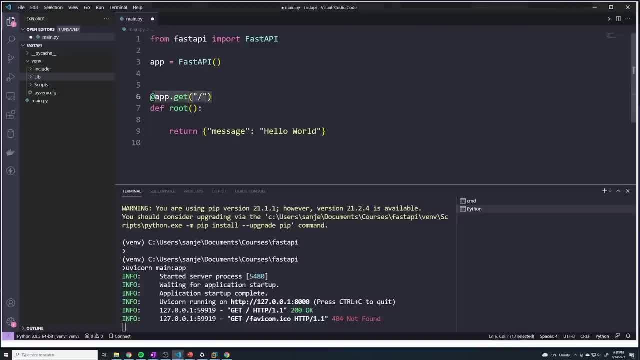 that on the web browser. Now the next thing that we have is this decorator. If you're not really familiar with decorators in Python, it's okay. You don't really actually need to understand. you know the core concept of a decorator. Just understand that when. 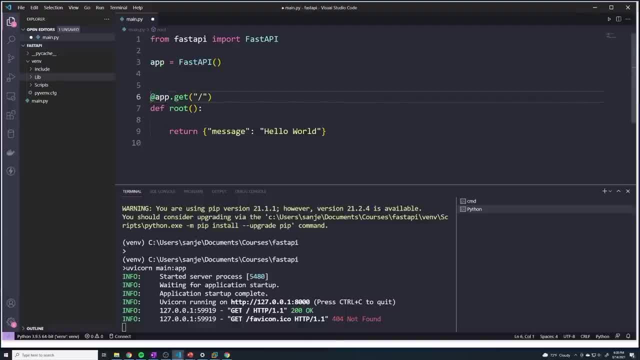 you apply a decorator to a function, it's going to perform a little magic to this function, Because if I remove this decorator, if we just commented out, take a look at this code. this code has nothing to do with fast API, it's a plain old function. So how do we actually make it? you know, act like. 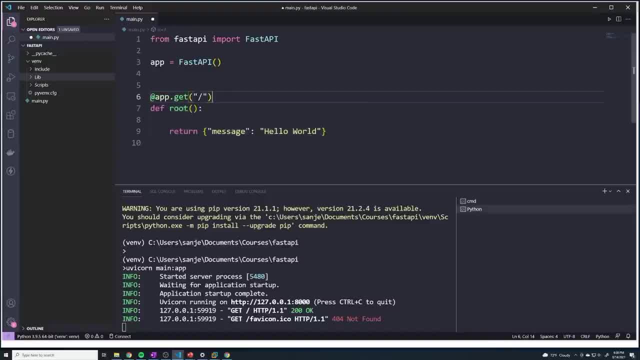 an API. Well, we have to use this magical decorator. This decorator turns this into an actual path operation so that someone who wants to use our API can hit this endpoint. And so you just specify at the at symbol: that's what the that's how we clarify that this is going to be a 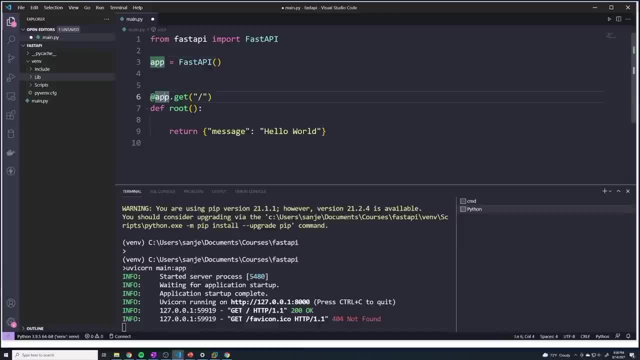 decorator, then we reference our fast API instance And then we have a couple of different options. So what here we pass in is the HTTP method that the user should use. So this is a get method, which means that we have to send a get request to our API, And. but we can use plenty. 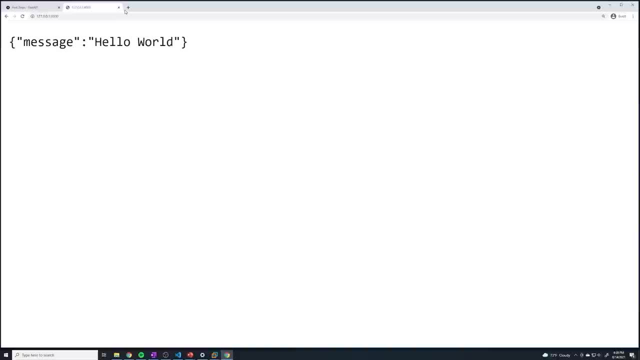 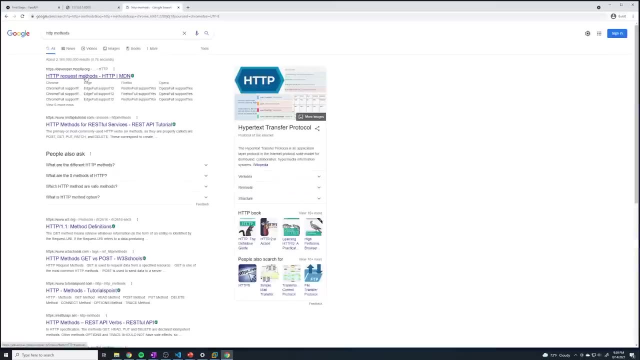 of different HTTP methods And I strongly recommend you actually take a look at the different HTTP methods. If you do HTTP methods, we can select this one. This is the Mozilla page. you can see all of the different HTTP methods. So there's get post put. 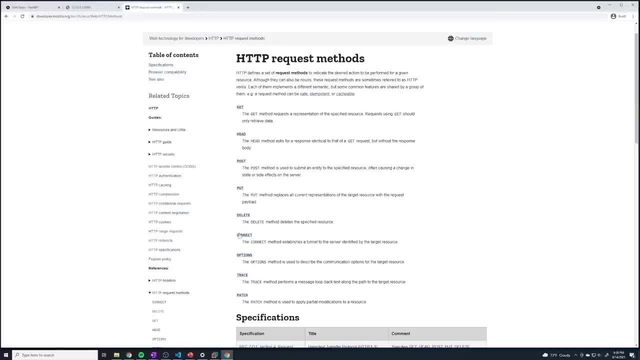 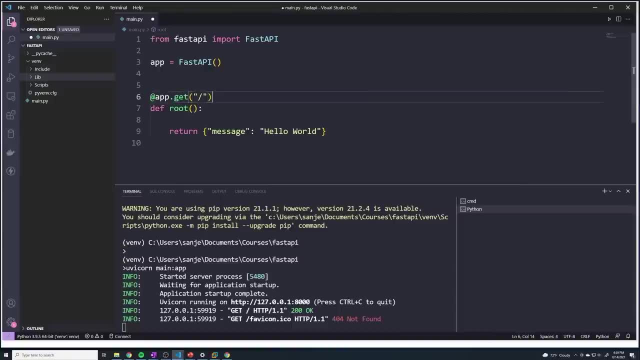 delete. So those are the main ones. There's a couple of other ones that are sometimes used, But for the most part those are the core ones, And so here's once again, just the HTTP method, And then, finally, we have the path, And so this is the root path, And so it's a little bit hard to explain the. 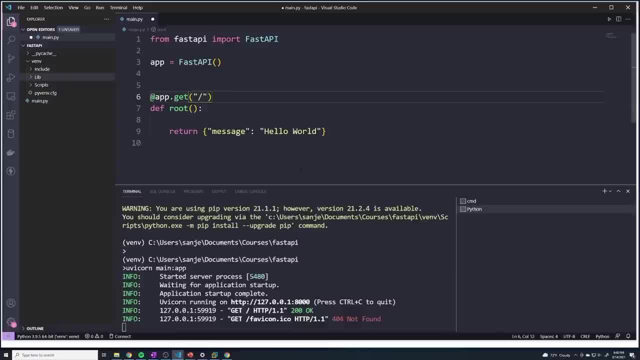 path, But it's basically the path after the specific domain name of your API. So if you take a look at our our URL, our web server is hosted on this specific URL. If I go to this page, let's open up a new link. 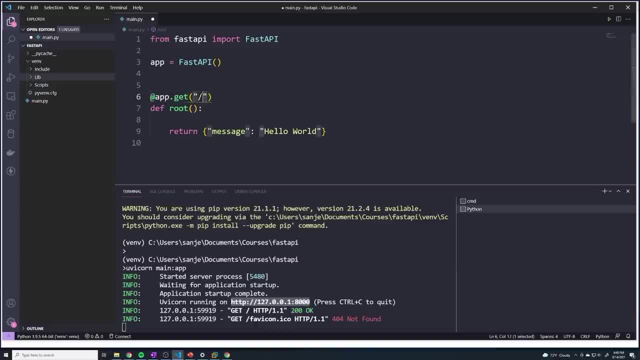 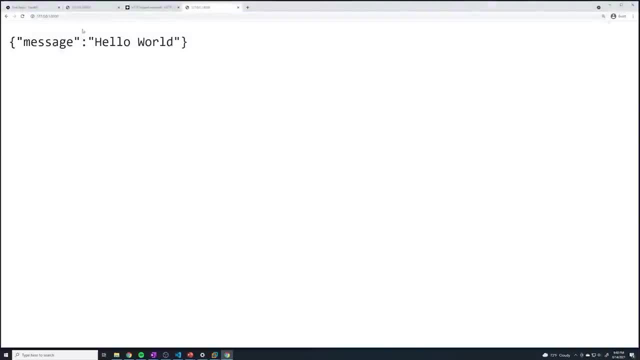 just paste it in here. So so the URL and the path in this case is just slash. So that's the equivalent of just hitting enter right here, or putting a slash which doesn't change anything. right, Right, whether the slash is there or not, it's basically going to take you to the same URL. 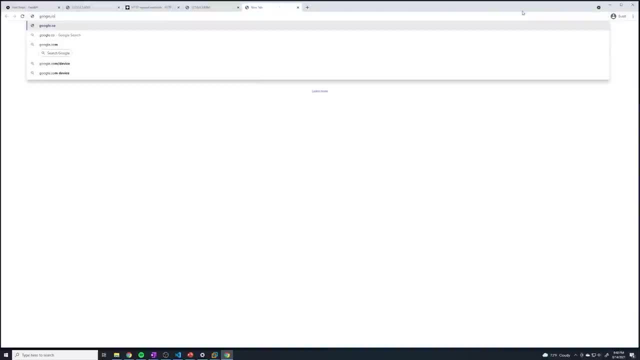 it's very similar to going to, you know, googlecom. Right, that's going to take us to googlecom, But if you go to googlecom slash it's. it's the same thing, So it's the root. 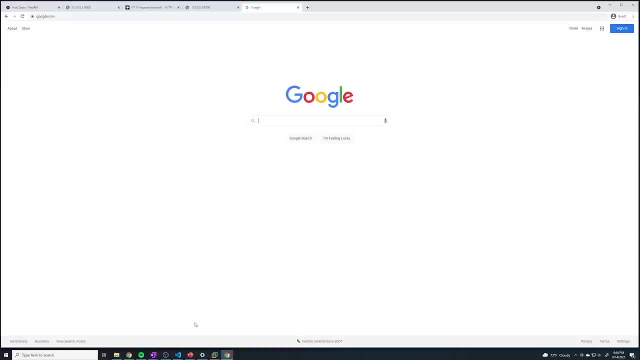 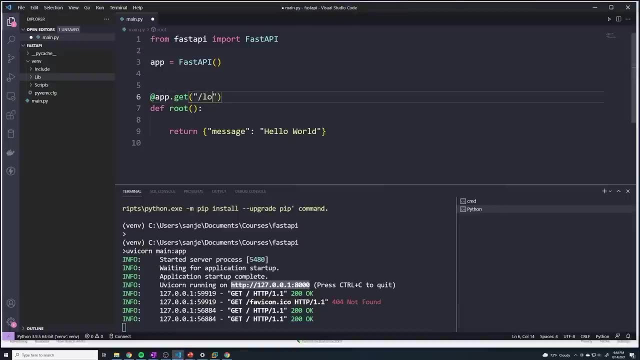 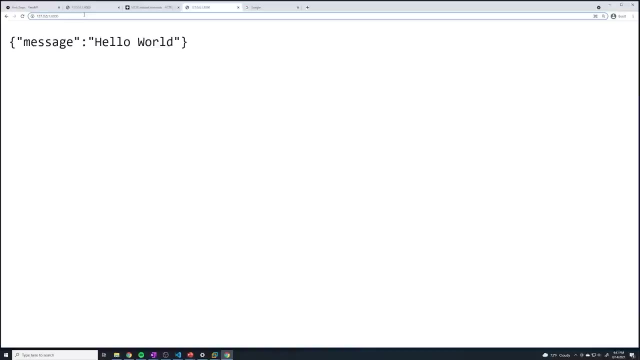 path. So whatever domain name our API is hosted, on, whatever URL, it's just saying it's the root path. You know, if I change this to, you know, login, right, that means that this path operation will only apply if the user goes to our URL and then goes to slash login. So that decorator, this. 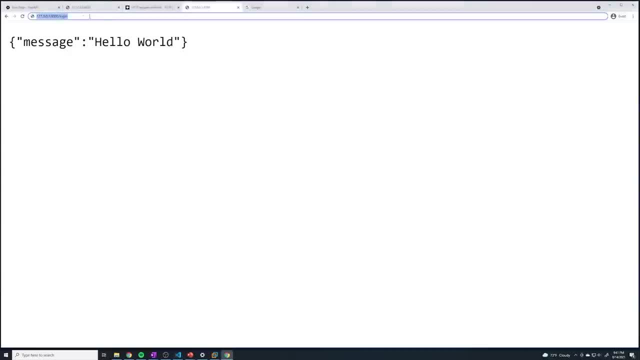 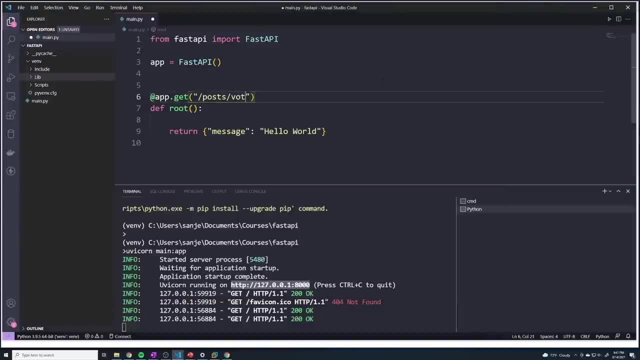 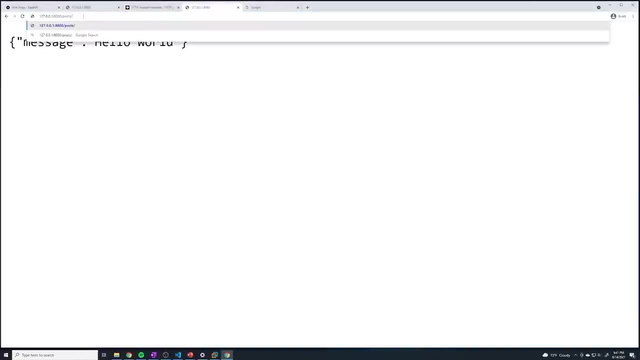 path right here just references the path that we have to go to in the URL, And so if this is actually changed to how about posts? and then you know, like vote, so maybe this is the URL for voting on a specific post- then we would have to go and do the same thing here, So we'd have to go to post slash. 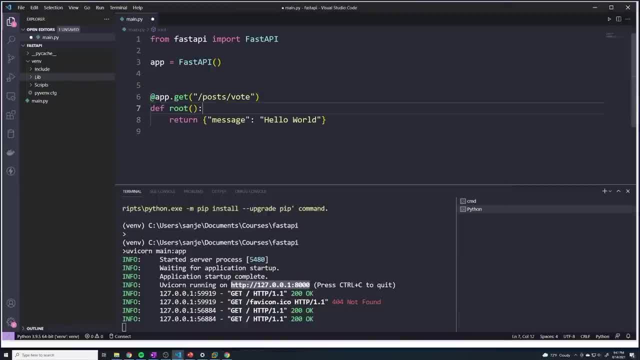 vote. So nothing too complicated, But those are the two pieces that make up a simple path operation. you've got the function, then you've got this decorator where you have to pass in the specific HTTP method and then the URL you want it to go to, And I'm going to change this back. 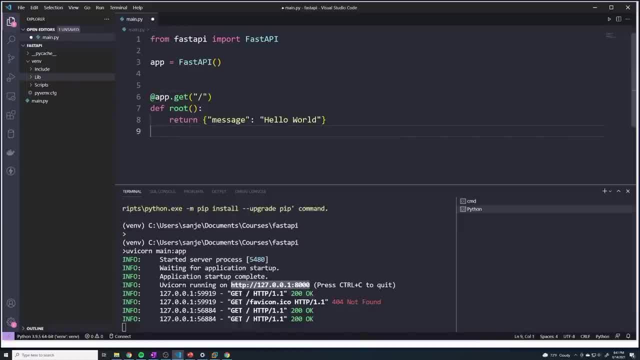 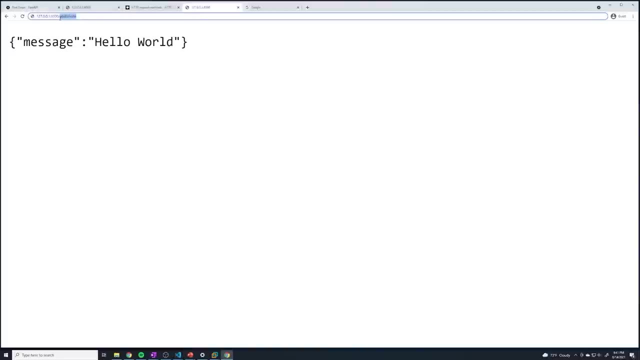 to the default. And now what I want to do is: let's go ahead and make a simple change. So what I'm going to do is I'm going to change this. I'm going to change the message to be welcome to my API. we'll save this. Go back to the root URL, because we changed. 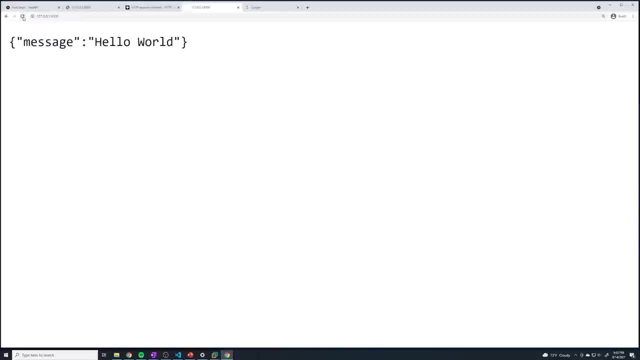 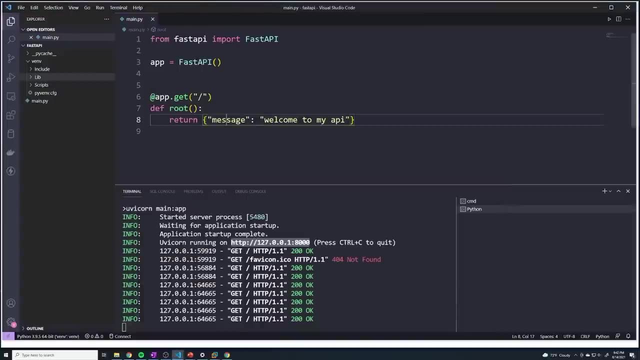 it to the root URL. Let's hit refresh. Notice how it still says hello world, nothing changed. So what gives right it? You know our codes changed. I saved it. Why are we not updating it so that it returns? welcome to my API. Well, the problem is: is that anytime you make a change, we 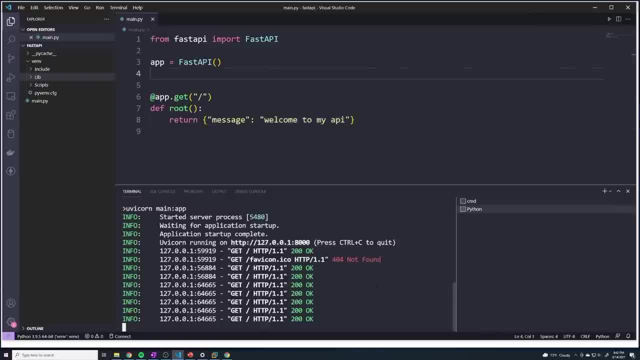 have to restart our system. So we're going to change the message to: welcome to my API. Let's do that server. So to restart our server, you hit control C, which is going to stop it. Then you could just hit the up arrow key so that you can find that command that you ran before and just run it again. 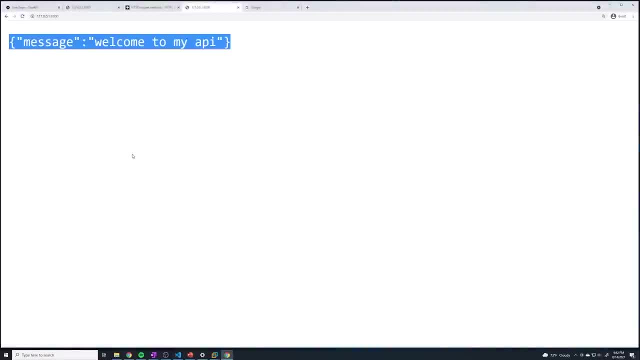 And so now, if I hit refresh, we can see that it updated. And I'm sure you're thinking: well, that's a little annoying. Every time I change my code I have to do a control C and then an up arrow and then hit enter. just that I can, you know, make sure that the server actually implements. 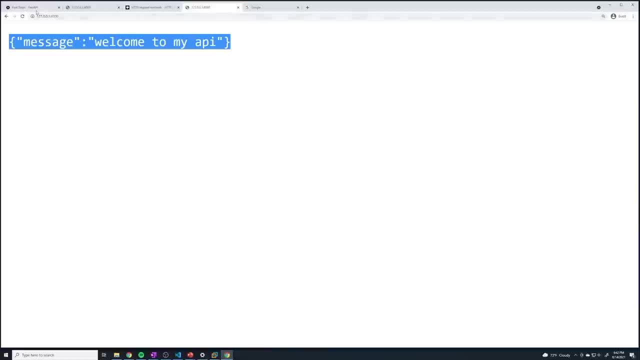 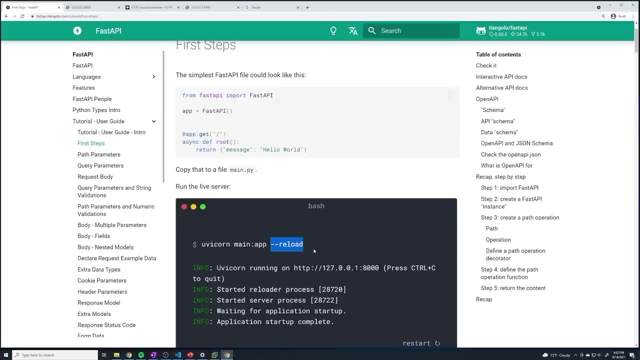 those changes And it is a little annoying but there is a workaround. So if we go to the documentation, you'll see that when they run UV corn they pass in the dash, dash, reload flag and the dash that reload flag will actually take a look at your code and monitor your code. So anytime, 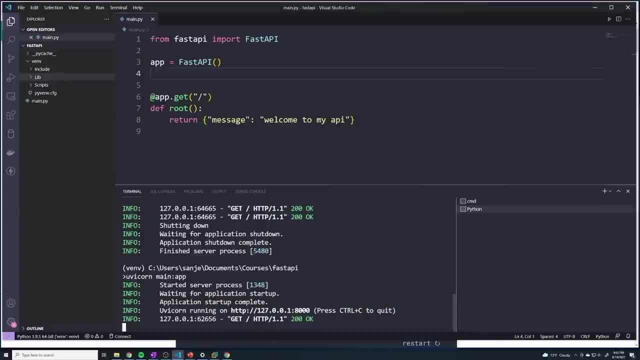 that you change your code, it'll automatically restart your server for you. So let's try that out. I'm going to do a control C, I'm going to hit the up arrow and I'm going to pass in the dash dash reload flag. So hit enter. And now what I want you to do is make some changes So it doesn't. 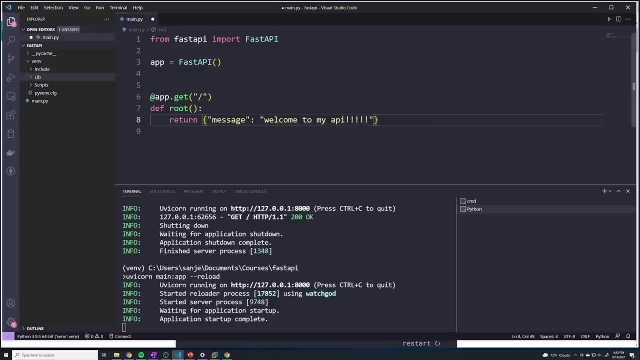 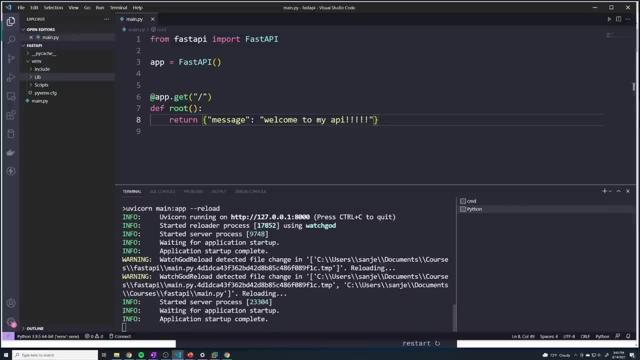 really matter what you change. I'm just going to add a couple of exclamation points and then I'm going to hit save And I want you to focus what on what happens down here. So if I hit save, look at that- It automatically restarted. 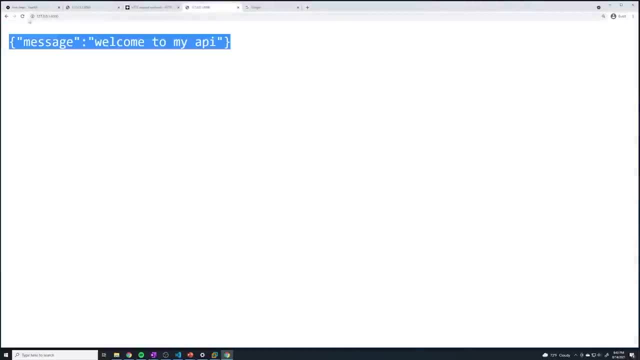 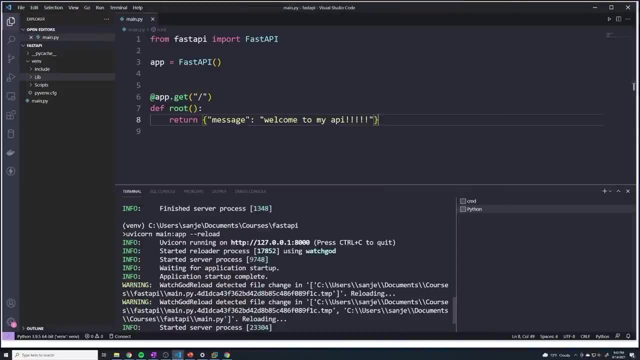 the server for me, And so now, if I go back to my website or my API, hit refresh, you can see that the exclamation points are there. So, moving forward in a development environment: only when we're in a development environment we're going to pass in the dash dash reload flag. When we go to 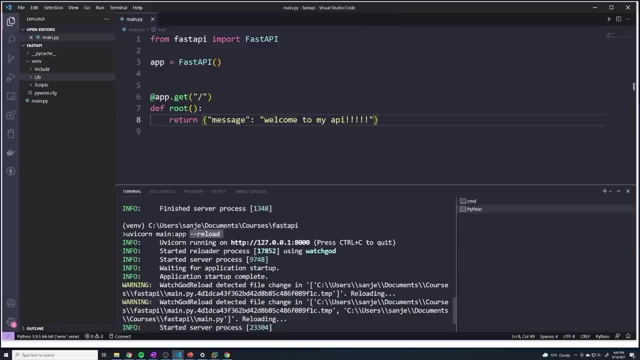 production. we don't need that. We're not going to be setting it up because we're not going to be changing our code in a production environment, And so I think that's a good stopping point here. Next video, we'll just quickly review exactly what is a path operation, so that we could just 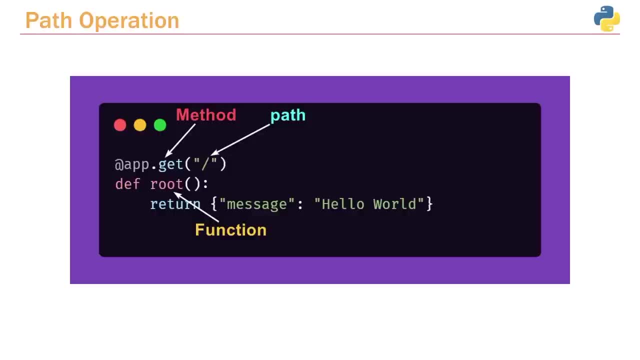 reinforce what we learned in this lecture. All right, guys, so let's quickly recap what we learned in the previous lecture. I want to make sure that you guys have a solid understanding of the different components of a path operation, because ultimately, that's all your API is. It's just a. 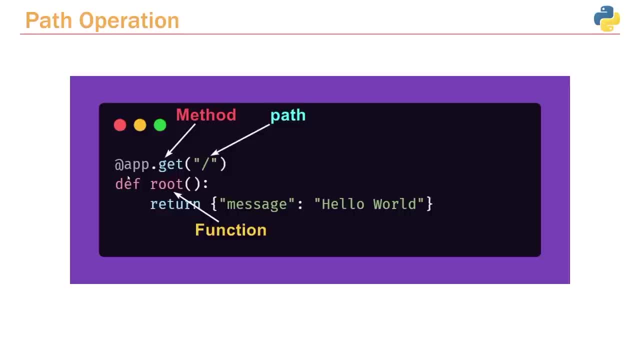 bunch of path operations. So first things first, we have our decorator. So our decorator has the little at symbol, And so that's what signifies it as a decorator. And then we reference our fast API instance, which we call our decorator, And so that's what signifies it as a decorator. And then we 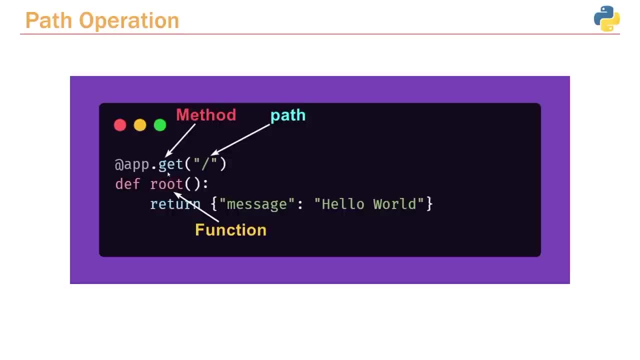 have our HTTP method. So in this case this is going to match only get methods, And then we have the specific path or the URL. So this is the root URL in this case, And then below that we've got our specific path operation function. So this function is going to contain all the logic for. 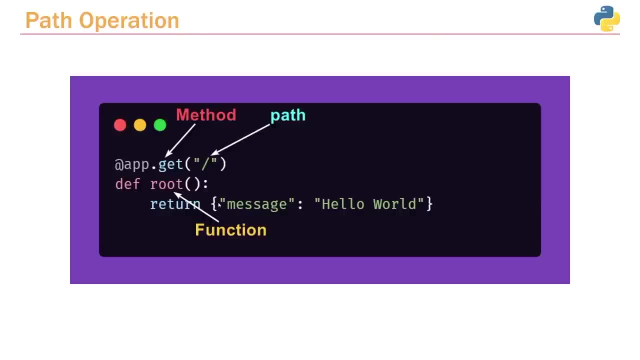 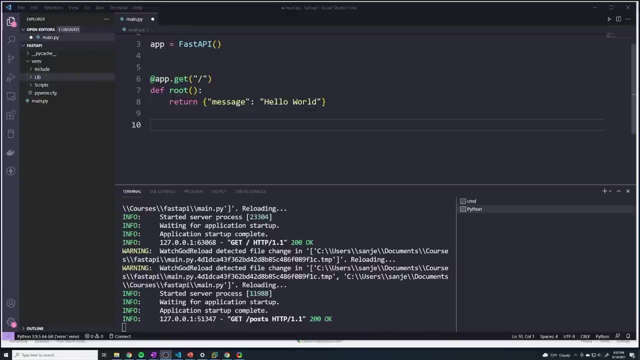 performing some kind of task And when it's going to return some data, and that's the data that gets returned to the user when they hit this specific path operation. So now that we have a solid understanding of how path operations work, let's see if we can create a new path operation And 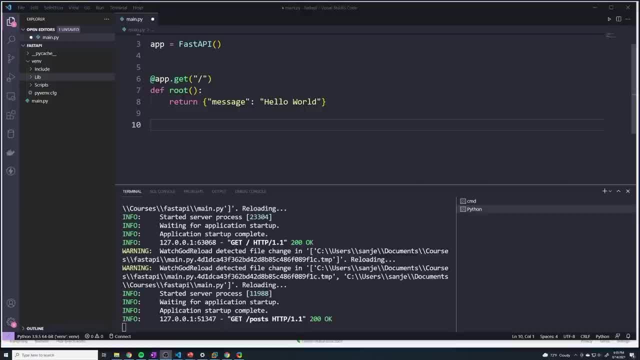 let's say, this one represents retrieving a bunch of social media posts from our application. So in this case, you know, there's two things that we need. So the first thing is our function, our path operation function. So we'll say def And then we'll give this function any name, I think, since 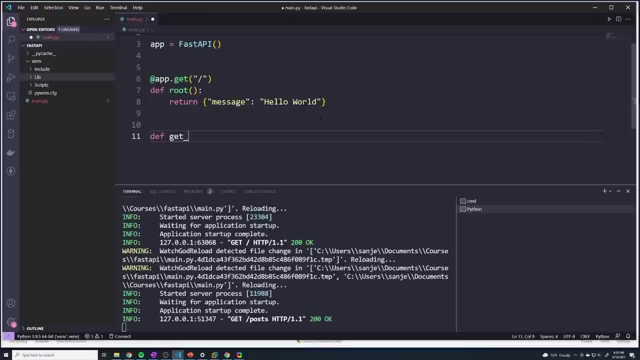 we're going to be retrieving a bunch of posts. I think a good name is going to be get underscore posts. But keep in mind, you can name this anything you want. Like I said, it does not impact the behavior of anything And then we want to see. So here we would pass in all of our logic for 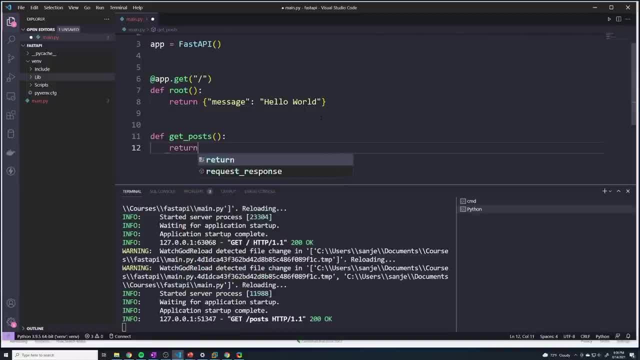 retrieving posts, but we don't actually have an application, So I'm just gonna say return And then we'll just say maybe I don't know data- And this is going to be: this is your posts, but in reality we would provide a list of posts, So let's save that. And then there's one last thing: we 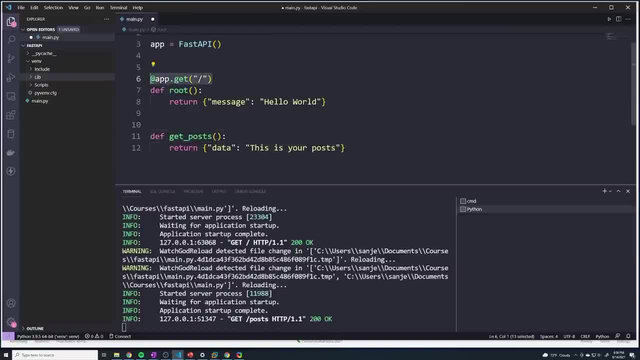 have to pass in our decorator, like we did before, to actually make this turn into a special path, path operation function. So we'll say at, and we reference the instance, the fast API instance, we'll do app dot, and then we have to figure out what HTTP method we want to use for this path. 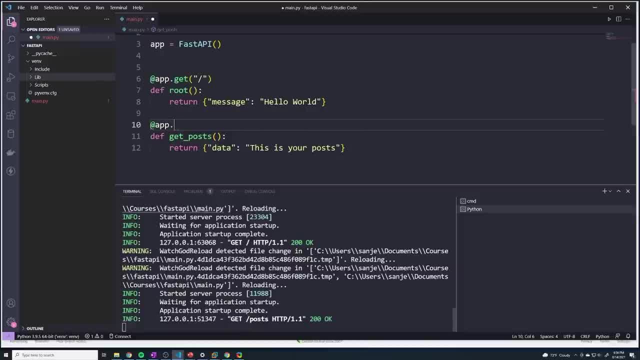 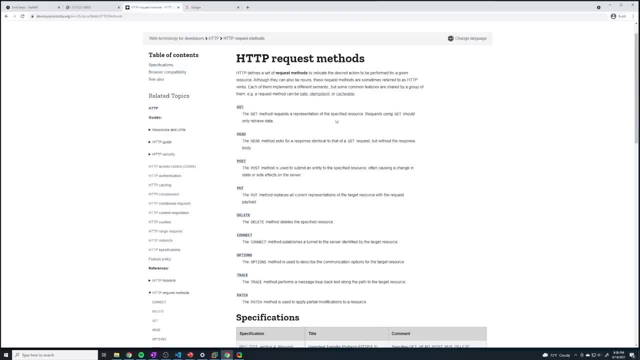 operation. So when it comes to retrieving data, you usually use a get operation And if you don't know which one to use, you can just go back to this page right here And it's going to explain what each one's for. So if you select get, it's going to explain when you would use a get If you. 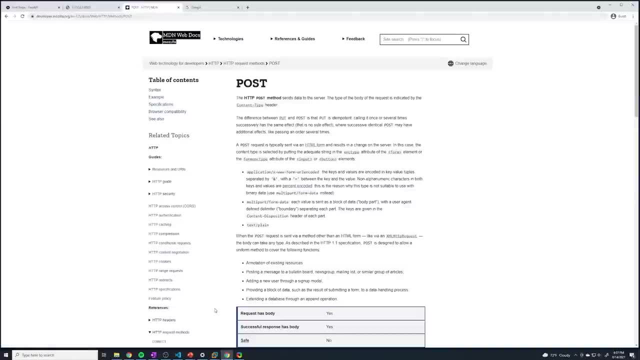 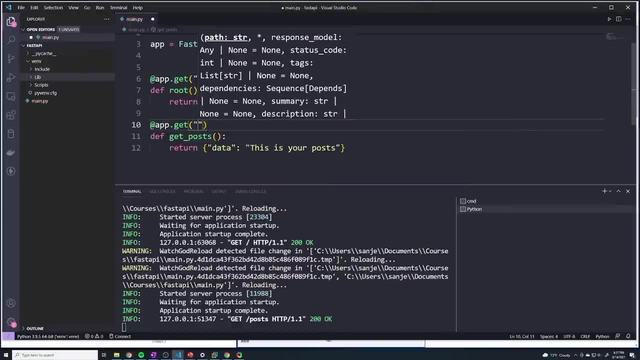 want to use a post. it's going to explain when you should use post, But I already know that for retrieving data it's usually a get operation, So we're going to keep it as a get method. Now for the URL. I'm going to say to retrieve posts. we want to go to the slash posts URL, So let's save. 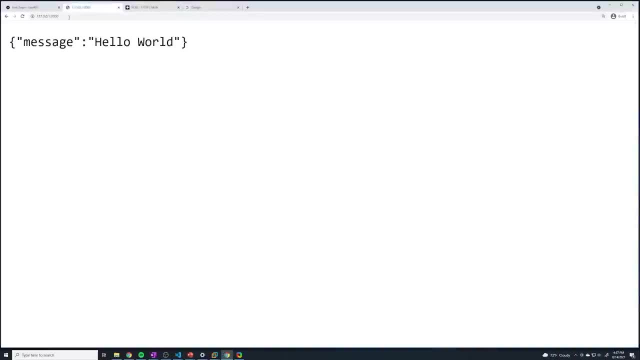 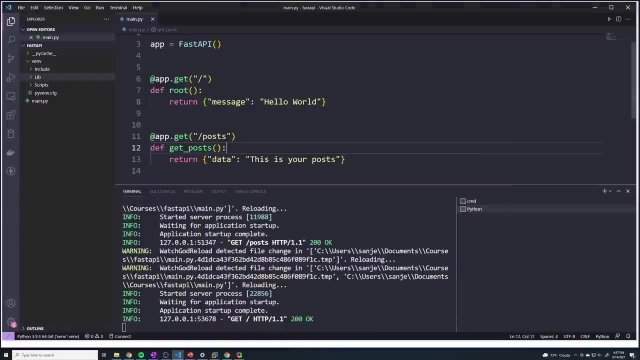 this And then let's see if we can retrieve that data. So if I hit refresh here, it's going to say hello world. But that's because if you take a look at this, we're at the root path And that's going. 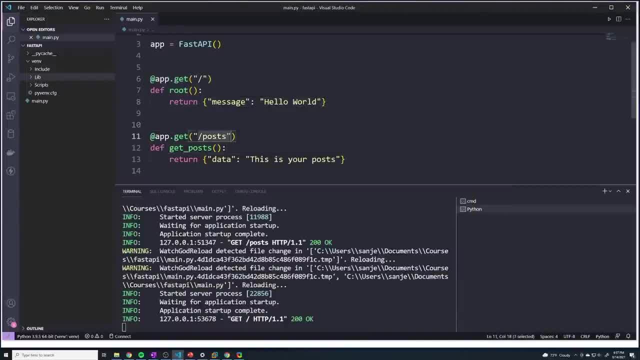 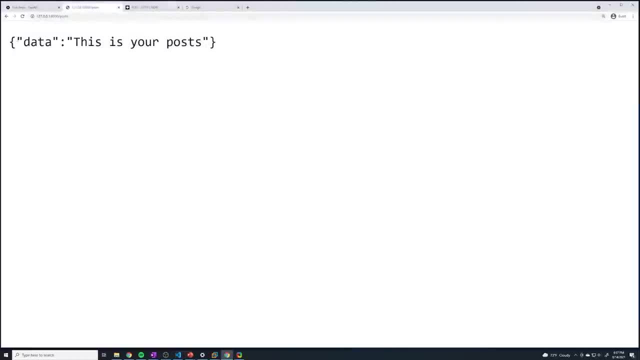 to match the data. So if I hit refresh here, it's going to say hello world, And that's going to match this specific path operation And this path operations on slash post. So if we go to slash posts and then hit enter, take a look at that. we have now got our data, which is our posts. So 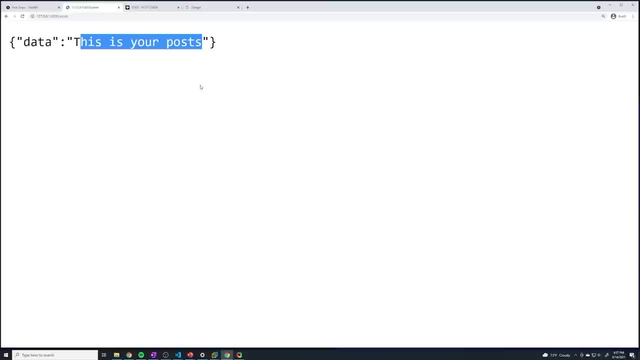 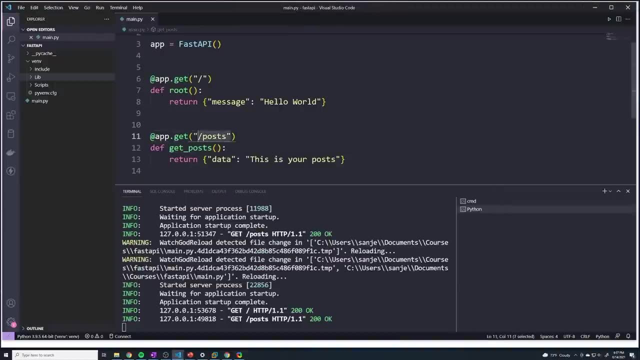 we've hit that second path operation that we just created, And it's really is as simple as that. you just define a function, you define the HTTP method and then the URL. Now there's one thing to know, And that is that you know the way that fast API works is that when, anytime, we send a request to 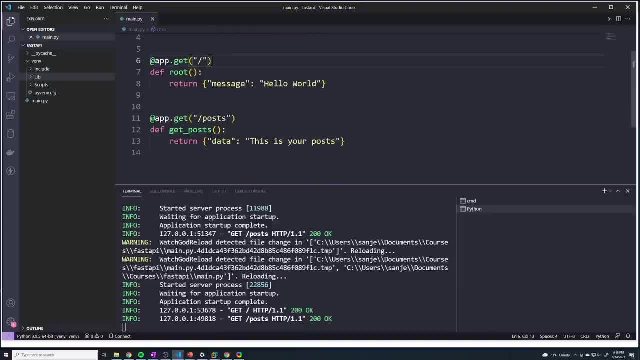 our API. we're going to be able to send a request to our API. So we're going to be able to send a request to our API server. it's going to actually go down the list of all of our path operations And then it's going to find the first match. And as soon as it finds the first match, it's going to 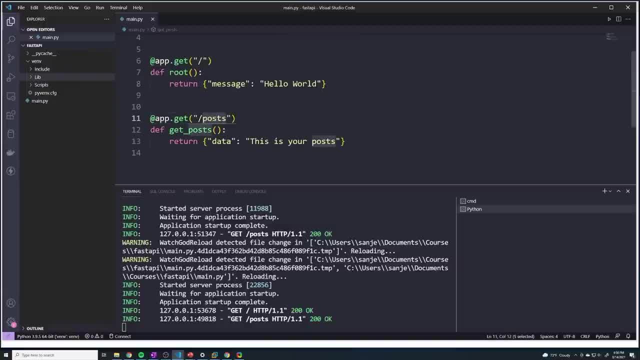 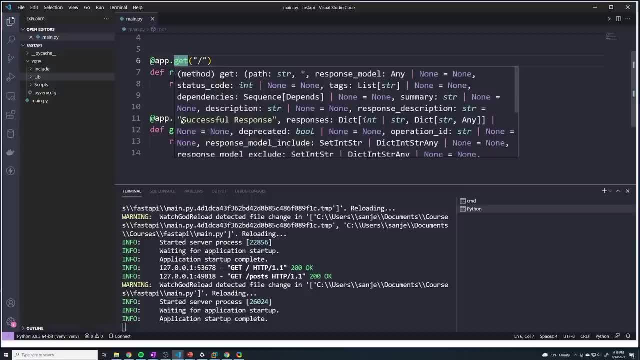 stop running your code. So if I actually change this to just the slash URL, just like this one above, what do you think is going to happen? Right, They both reference the get method and they both reference the same URL. So which one do you think is going to win? Well, let's take a look. 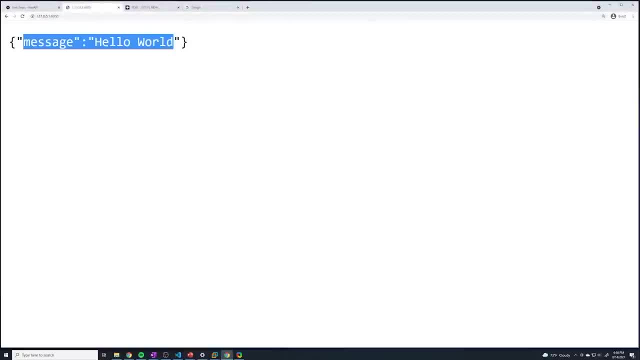 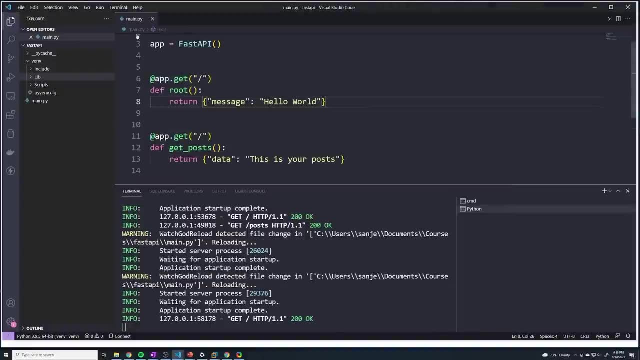 If I do just the slash again, it says hello world. So it looks like the first one one, And the reason for that is that once again, fast API literally just goes to the code and it looks for the first match. So there's really only 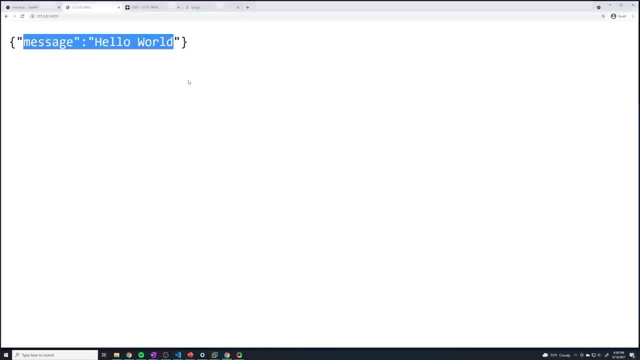 two criteria in this case. What's the HTTP method? It's a get. So anytime you work in your browser, your browser is always going to send a get method by default. And then what's the URL? So the URL is a slash URL, So it matches this one And it does not continue past that, So it never runs this. 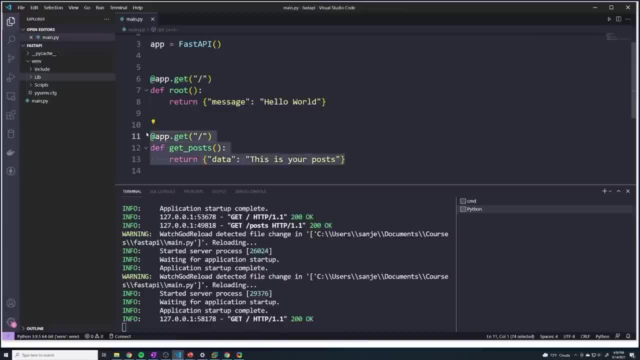 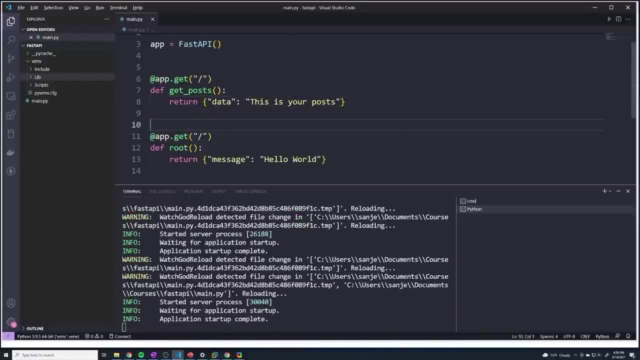 code. So it sends that back. Now, if I took this, copied it and moved it to the top, what do you think is going to happen? Which one do you think is going to run? Well, let's hit refresh. Look at that. So that one ran. So the first path operation that matches is always going. 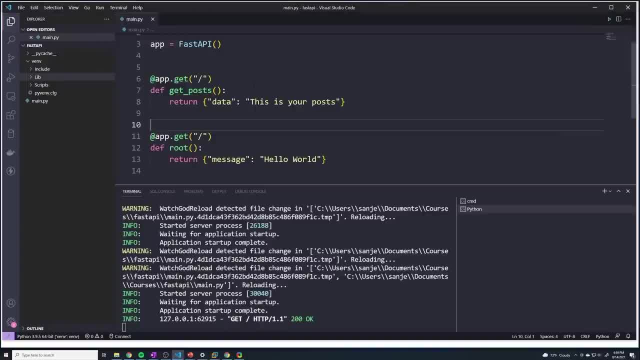 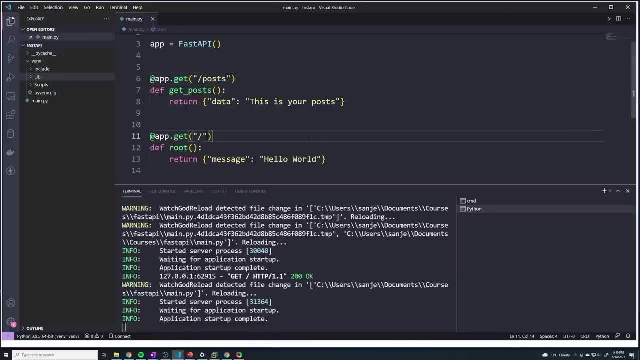 to be the one that runs. Simple as that, So the order does in fact matter. However, if I change this to posts and leave this at the top right, if I hit refresh, we get hello world. So what? 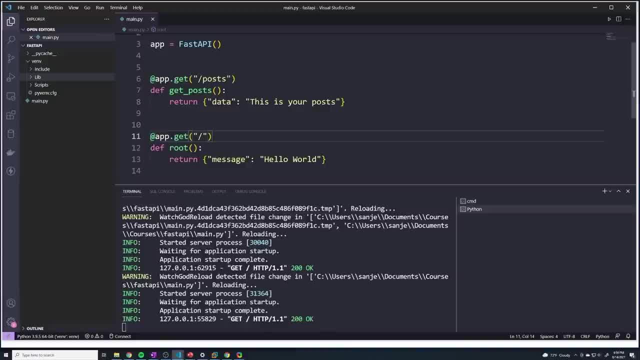 happened was fast. API went down the list right And it received a request That. let me just put some comments. So the request comes in. Sorry, that's not the way to comment. in Python, Request comes in with a get method And it comes in with the. the URL is going. 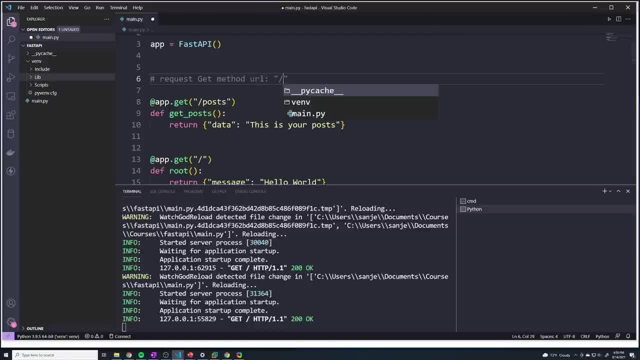 to be slash, All right, And so these are the two things that it looks for to match. So it hits the first path operation, So this is a get, So those two match. And then it looks at the URL, which is slash, But that does not match. So it skips past with this one And then it goes to the next one. 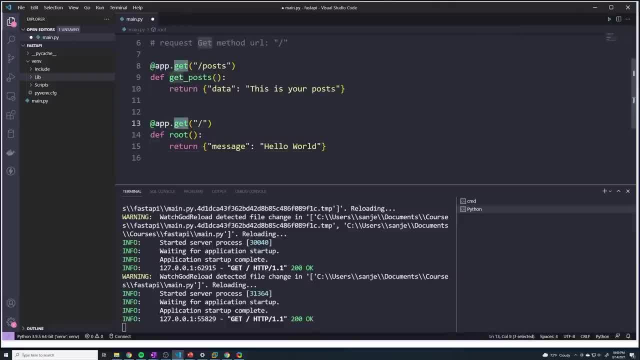 And then it checks to see if that matches, So then get matches, the URL matches, So then it returns hello world. And that's why it returned hello world. And the reason I wanted to highlight this is that the order in fact does matter, So you have to keep that in mind And it can impact the 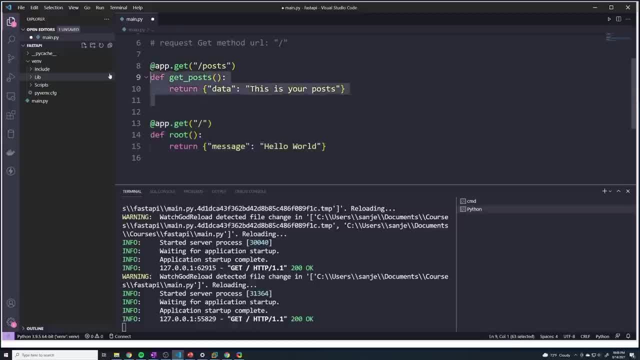 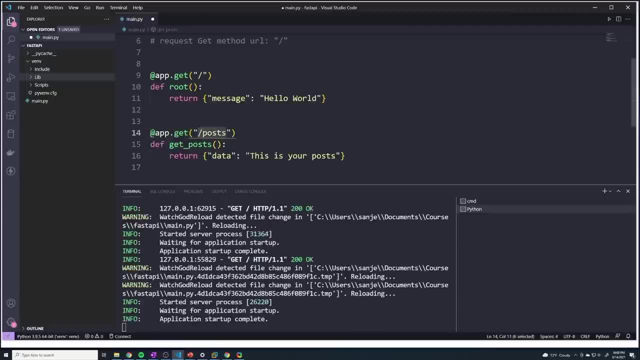 way your API ultimately works. I'm going to just take this, move this to the bottom, But in this case the order doesn't matter, because they're hitting two different paths or two different URLs. So that's the order, And then it checks to see if that matches, So then get matches. The URL matches, So then it. 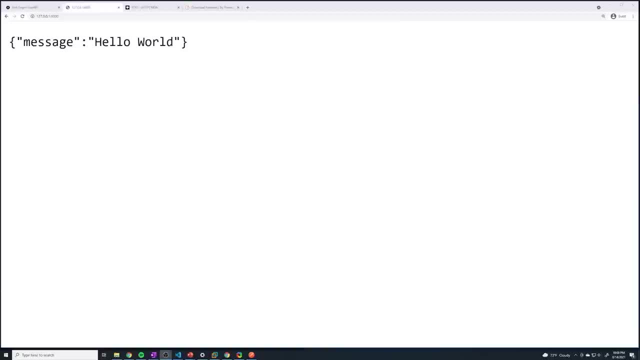 We've been using our web browser to generate HTTP requests to test our API, And that's fine for now. However, once we start getting into more complex path operations and routes- so things that involve having to send a HTTP put or patch or any of the other methods- and having to send data to our API, 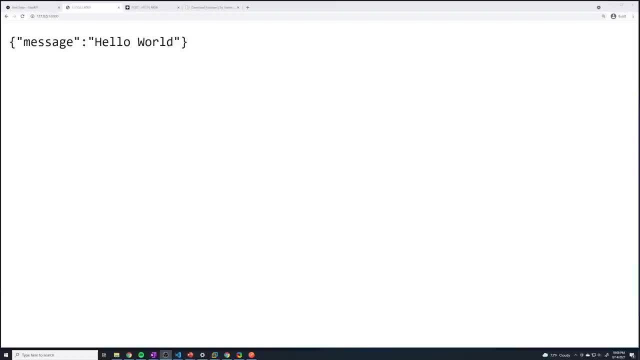 it gets very complicated because there's no way to natively do that in the browser without generating or building out a complete full front end application And to test an API. you shouldn't have to build an entire front end application to do that. 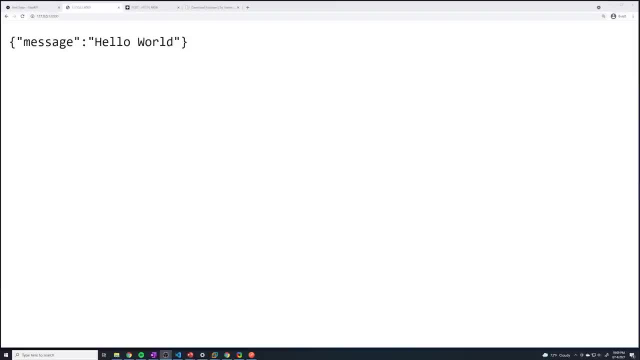 That would be, you know, unmanageable, unscalable, And so there's a lot of different tools that we have that we can use to test our API, And so one of these tools is called Postman. If you go to postmancom slash downloads, you can download this app, So go ahead and just hit. 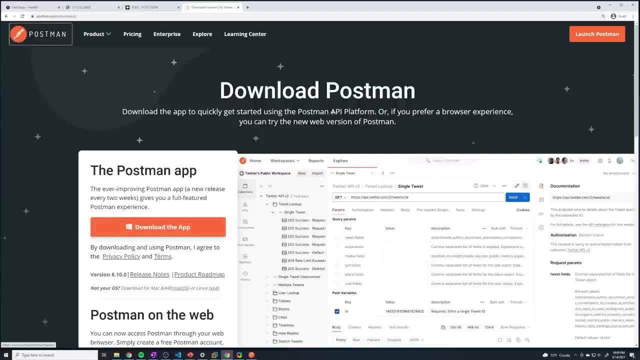 the download button. it's going to automatically detect what your operating system is. But this is a very simple tool. It's just a tool that allows us to construct our own HTTP requests. So we get to specify the individual fields of an HTTP request. So we could. 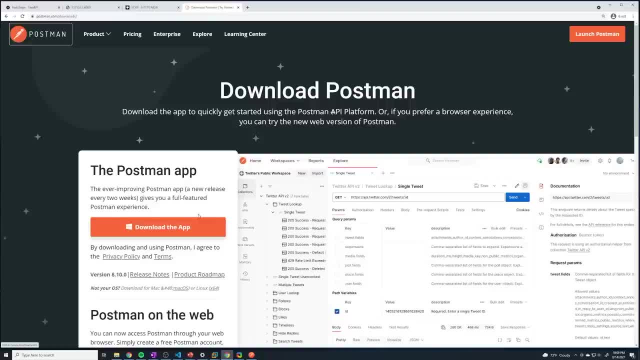 specify. you know, what is the HTTP method, What's the URL, What are the headers that we're going to apply, What's the body? What kind of data is that going to carry? Is it going to have any authorization headers? So all of these things we get to construct in a nice GUI so that we can test. 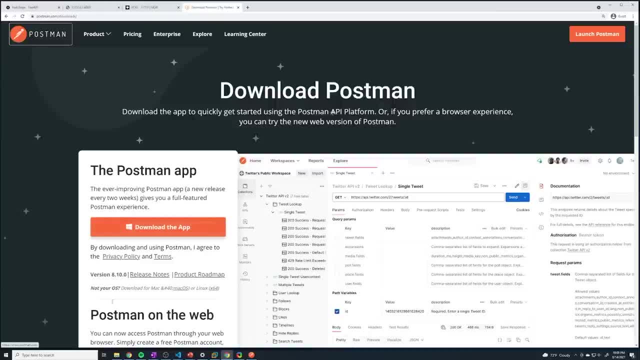 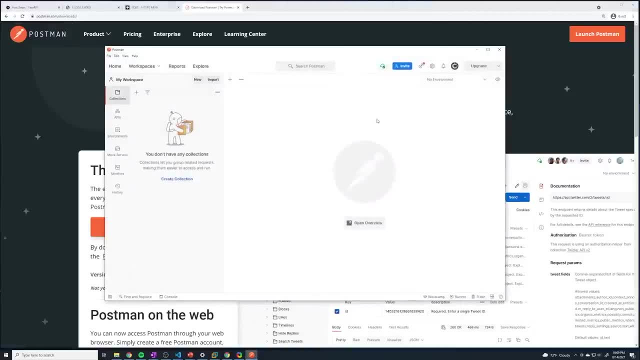 our API. So go ahead and download this Now. I've already got it downloaded. But once you've got downloaded, open up the desktop application And you should see something like this: right. Everything is relatively empty, And what we want to do is, if we want to create a new HTTP request, all we have. 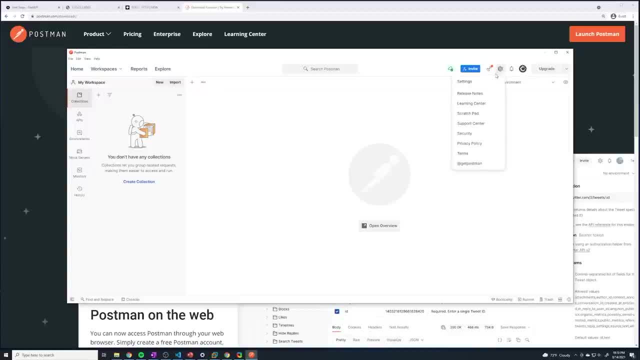 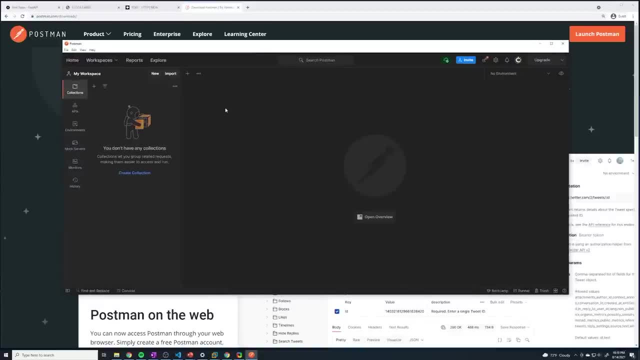 to do is hit the plus button, And before I do that, what I'm going to do is: let's change this to dark themes, So themes. I think this looks a little bit better. Yeah, that looks a lot better, And I'm also. 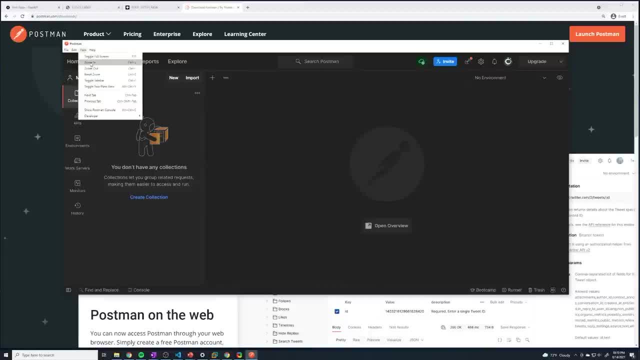 going to zoom in for you guys. Let's make it a little bit more. There you go. Hopefully that's nice and easy for you guys to see now. So what we want to do is let's create a new HTTP request. So 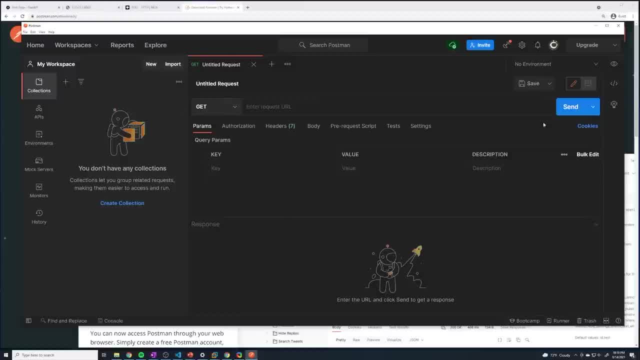 hit this plus button And you could see that this provides us all of the fields that we need to actually create an HTTP request. So the first thing that we need to do is specify what's the HTTP method. So if we go back to our code, 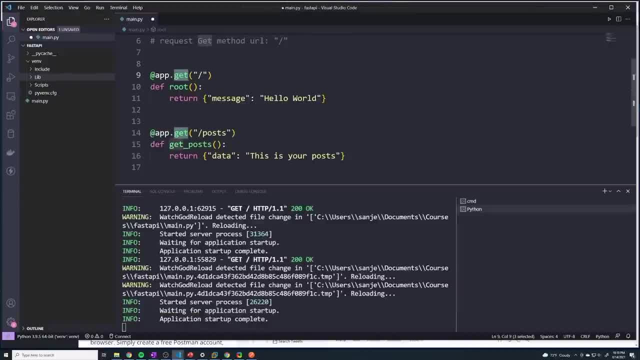 right, we only have get requests. So whether we want to hit either one of these path operations, it's going to have to be a get request. So we're going to leave it as get. but you can see, we have all the other whoops, we have all of the other options. then we have to specify the URL. So this: 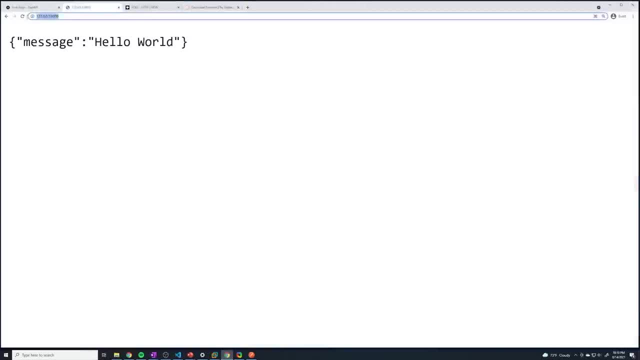 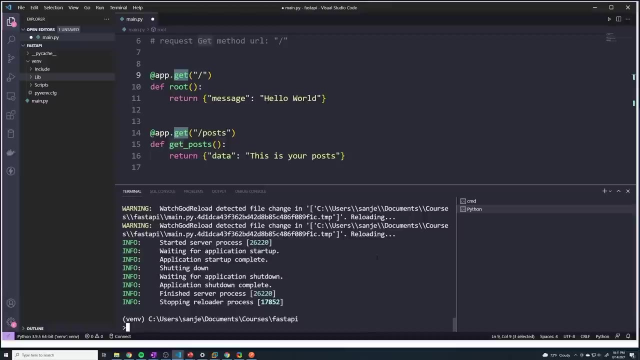 is no different than the URL that we went to in our browser. We just copy this URL And we actually need the HTTP in there as well, probably So, if we actually go back to our server and see where we started it and actually the best way to get the URL is just to stop it. 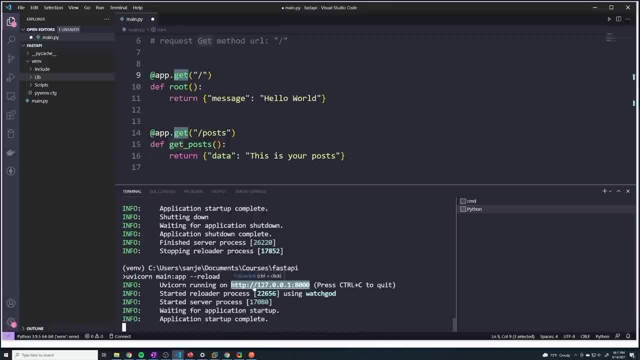 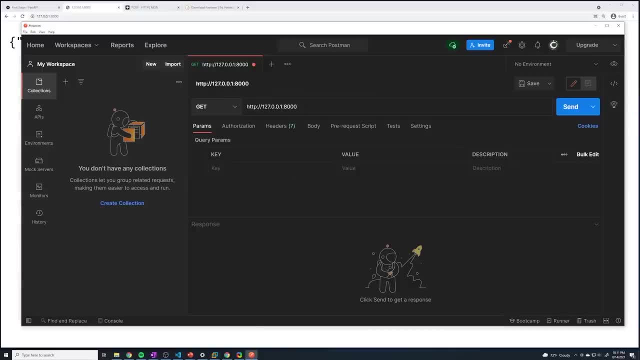 start it And then that's going to give us the URL. So we just needed the HTTP beforehand And then we just paste that in there. Okay, and so if I leave this as the you know the route path, whether I include the slash, it doesn't really matter Actually. 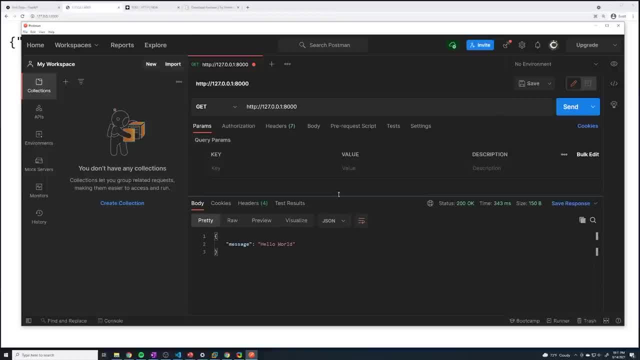 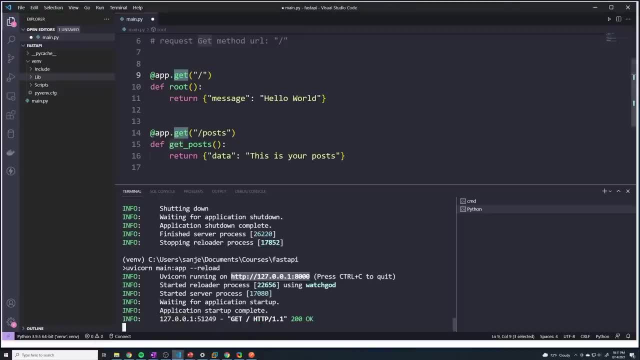 we can just hit send And you look at this, this is the result that we got back from our API server. So it says message: Hello world. And once again, you guys already know where that came from And that came from this specific return statement, And so you could see that this is so much easier. 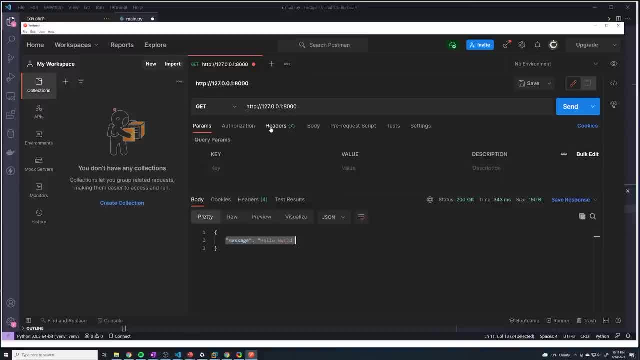 than using a web browser. Well, you guys may not notice how easy it is at this point, But once we get to constructing more complex path operations, you'll see that it's so much easier to use a tool like this. And keep in mind, this isn't the only tool that does this. there are. 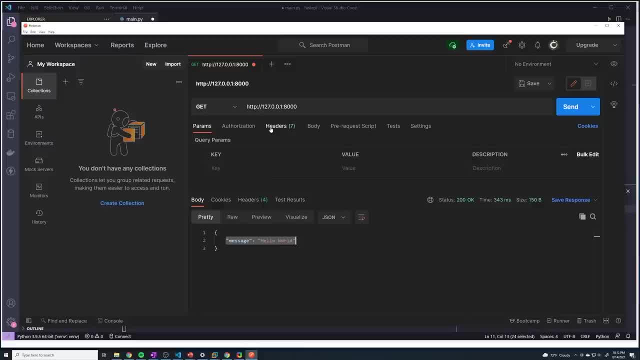 other applications that also do this. this is just the one that I'm familiar with and the one that I use, But I don't want to, you know, force any specific application down your throat. you guys can use whichever one you want. So if you already use one that you prefer, feel free to stick with. 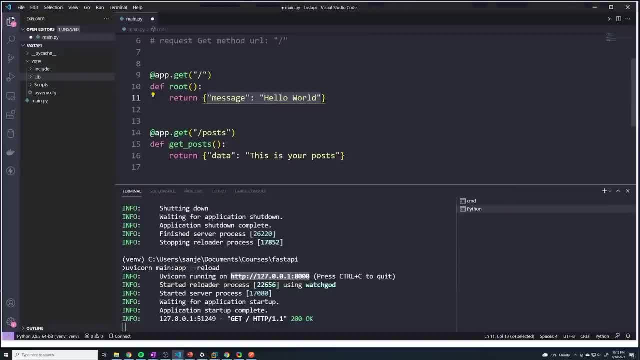 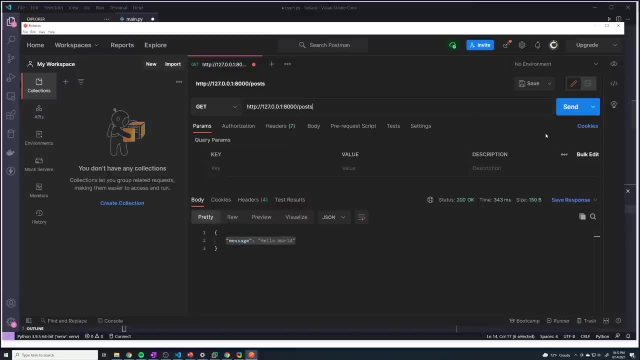 it. But before we wrap up this video, let's just test out our other specific path. So this one's going to reside on slash posts. we're going to try that and we'll do slash posts. We'll hit send And look at that. we got our data that says this is your posts. So now we were successfully able. 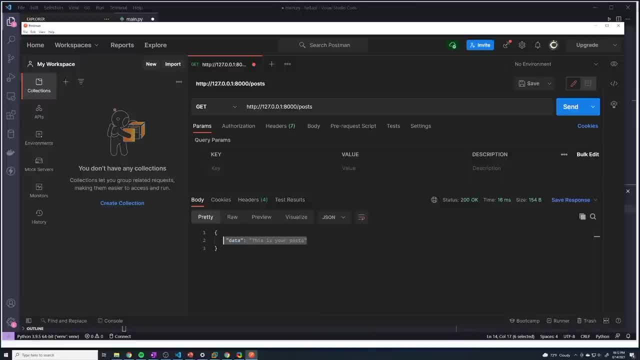 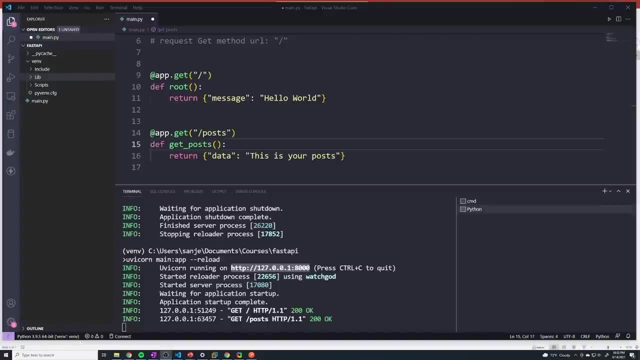 to test out both of our path operations using postman And moving forward for the rest of this course. we're no longer going to use the web browser. we're going to use postman to test out our API. Till now, we've only been working with get requests, So all of the HTTP requests we've 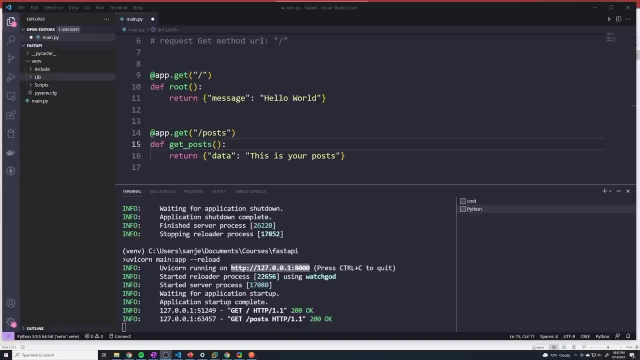 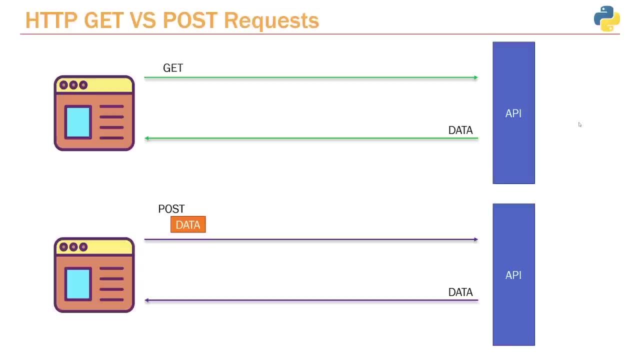 sent to our API. all have been get requests, And so now we're going to learn about post requests And they're a little bit different, And I want to kind of highlight what makes post requests different than get requests And I've drawn out a little diagram for us. So at the left side we've got our web browser. 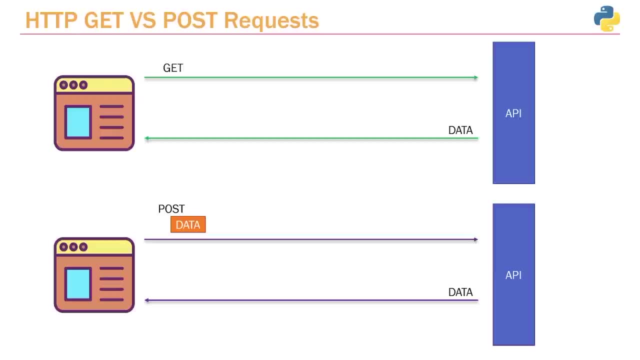 or it could be our mobile device, depending on whatever the front end is, And on the right side we've got our API server. So this is our fast API server. Now with a get request. what we do is we just send an HTTP get requests And then we send that to our API server, And then our API server. 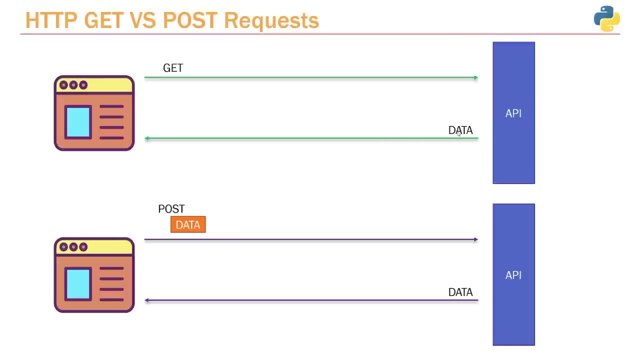 sends back some kind of data, depending on what they're trying to get. So if they're trying to get a whole bunch of posts, we send back the posts. Now, with a post request it's going to be different And that is that with a post request we can send data to the API server. So in this, 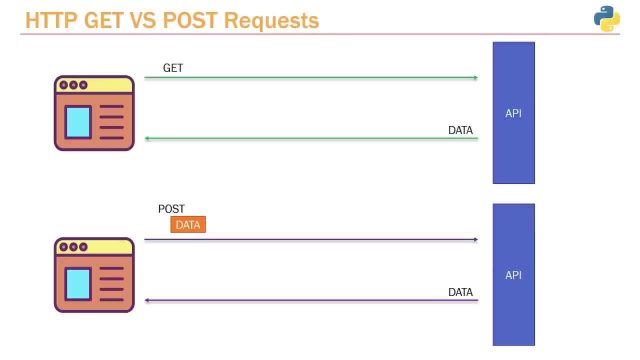 case. a lot of times, what you'd use a post request for is for creating things. So if I want to create a post, I would. when I say post, I mean like a social media post, not post as in post request. 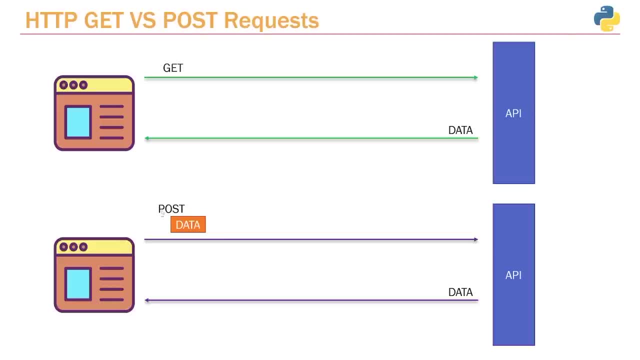 But if I wanted to create a social media post, I would send an HTTP post request And I would include all of the data needed to create a post on my API server. So we'll send that data over to the API server. The API server will send back whatever data it thinks it needs to send. And so in real life, if we 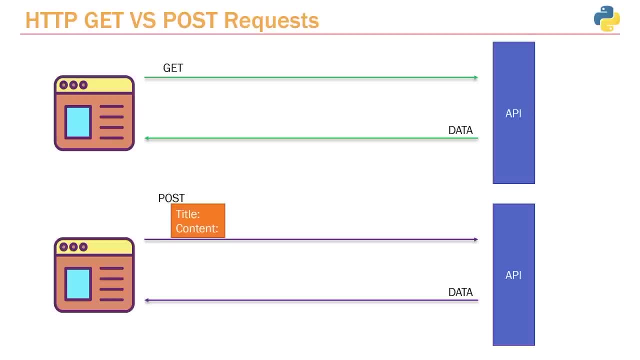 were trying to create a post, we would include whatever data we needed for a post. So in this case we would include what's the title of the post, what's the content of the post, what's the user of the post. we send that to the API server. The API server can then talk to whatever database. 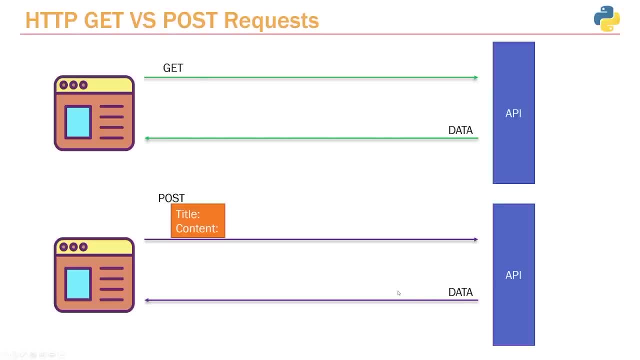 to actually create the post And then it can send back some data. you know something like: hey, I've successfully created the post, And then here's the final post, after I create it, and then send those details, And then it can send back to your web browser or your mobile devices. So think of it like this: a get. 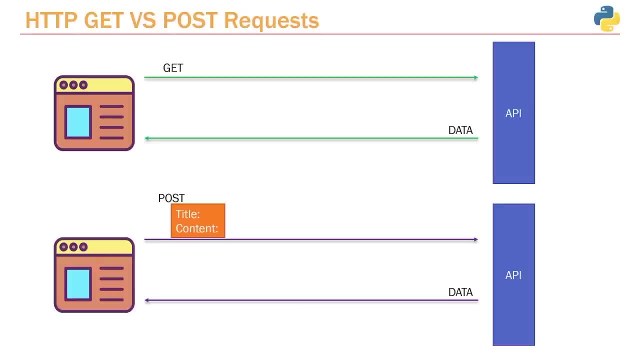 request is basically saying, hey, API server, give me some data, Whereas a post request is saying, hey, API server, here's some data, do whatever you need to do with it. So it's like: so it really controls the direction of flow of data between the front end and the API server, So get requests. 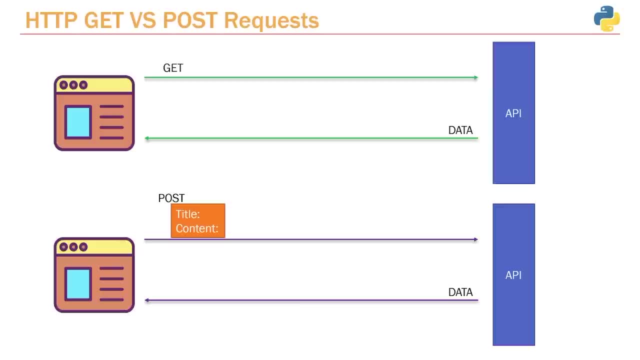 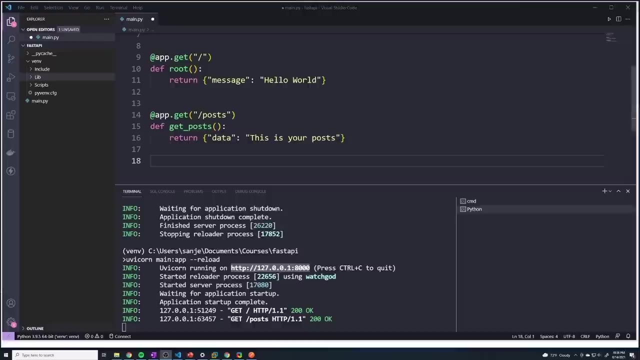 are getting data from the API server, whereas a post request is sending data to the API server. So now that we have a basic understanding of how post requests work, let's go back to our code and see if we can create a path operation for a post request. So let's go below our last path operation, which was forgetting. 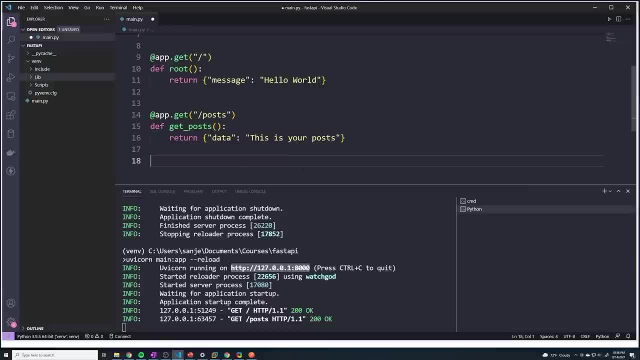 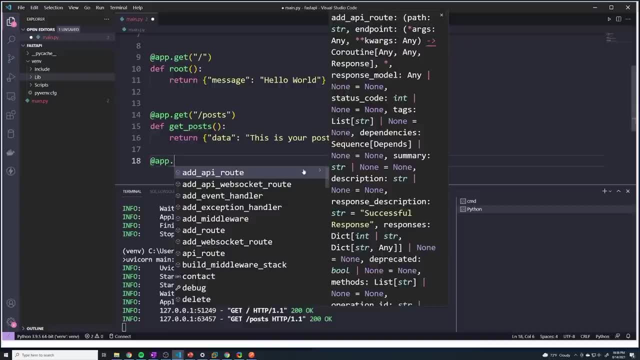 posts And let's create one for creating posts. So, first things first, let's, let's just actually create our decorator First. we'll do app dot And instead of guest- sorry, instead of get- we're going to say post. So that's all it takes to convert a traditional get request to a post. 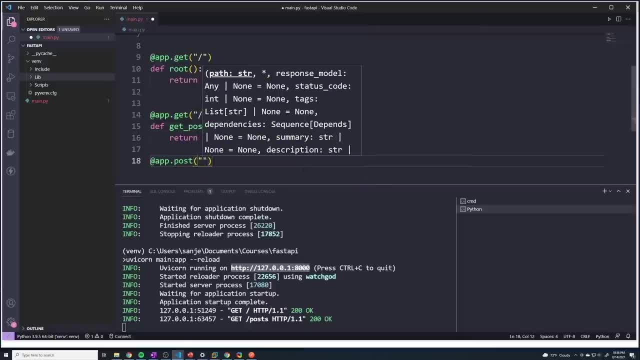 request, you just say dot post And then, once again, we're going to say whatever specific request we want to create. So we're going to say dot post And then, once again, we're going to say whatever specific URL the user should go to to actually create the post. Now I'm going to do something a little bit. 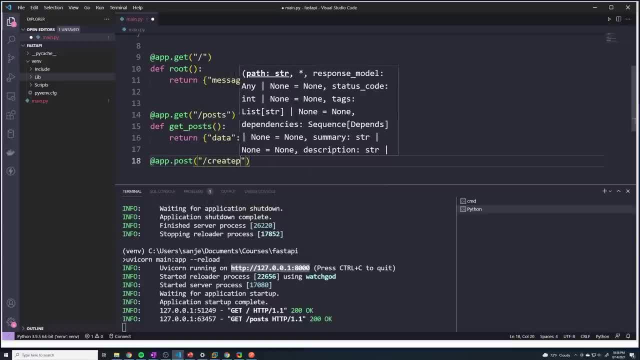 bad. I'm going to say the path that we want to go to is called create posts, And if you've ever worked with API's, this is kind of going against best practice. But don't worry, we'll correct this in the next lesson Because there are certain best practices. it's not going to break our application. 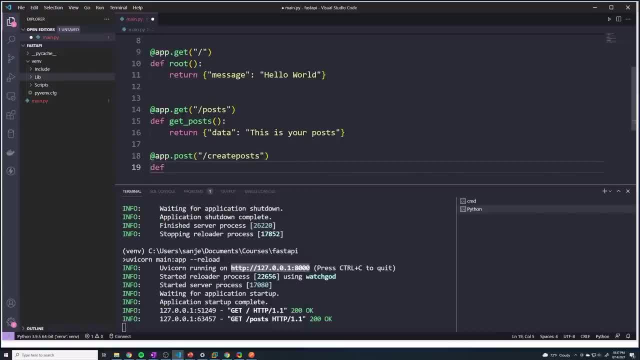 by any means. We'll say this, and then we'll say def. And then here we'll just name our function. I'll just say create post. Like I said, the name of the function never matters. And then here which? 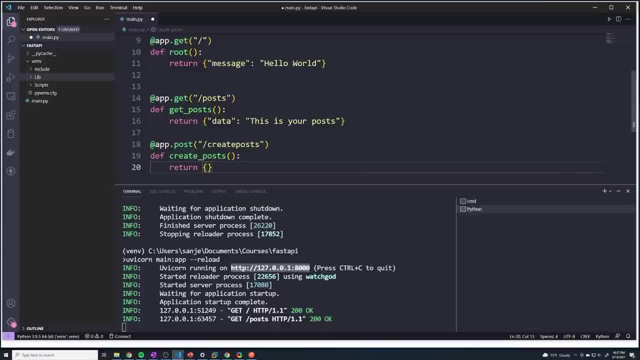 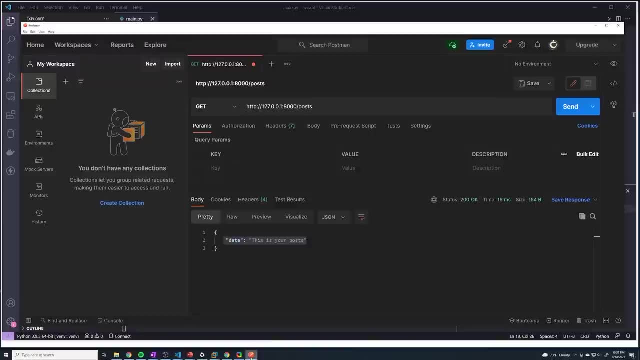 we're all we're going to do is we're going to return. we'll say message, whoops, message. And then we'll say successfully created posts, Let's save that And let's go to our postman. And so we've got already one request, So I could just change this to post, And then we have to change. 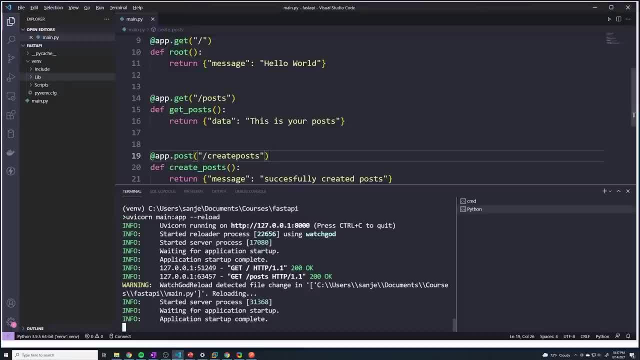 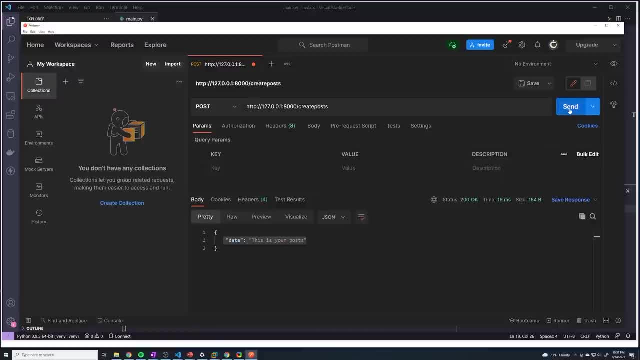 the URL in this case. So we'll go back and see that create post. So it's going to be at create posts And let's hit send And let's see what happens. Look at that message: successfully created. So we have successfully sent a post request to our API. Now one thing. 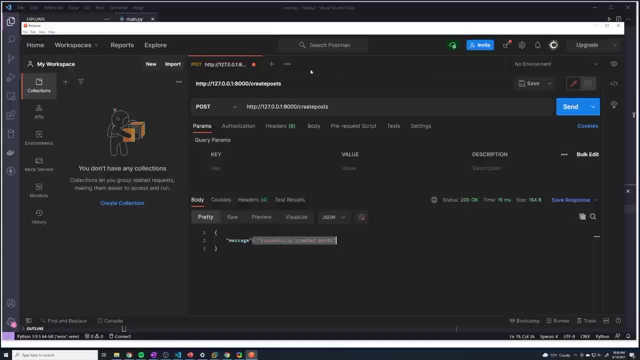 I like to do with postman is that you can create multiple requests and then have them saved. So I'm going to actually change this back to just go to post and then go to get, and then we'll keep that, and what we can do is we can just add another request, And so I'm just going to copy the. 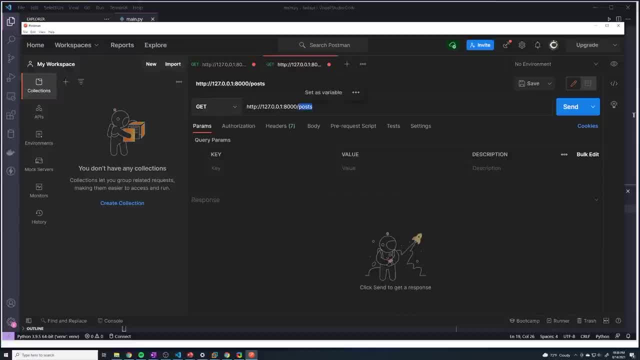 URL here I'm going to paste this And then this is actually going to be create posts And then this could be a post request, And so now we can hit a get request and then hit a post request really quickly, Because they're essentially we've got them in two different windows. 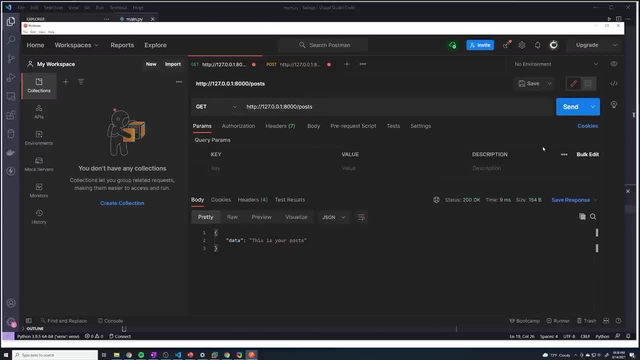 And let's just quickly double check that still works, That's good. And then let's double check it: get post, that still works, Perfect, Now, that's cool and all. However, the whole idea behind a post request is to send some data. 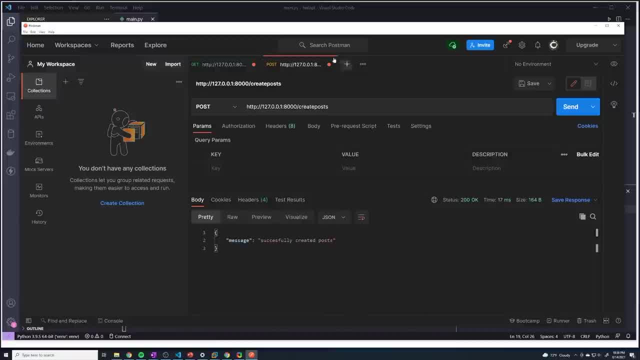 to our API server. So we're going to go ahead and create a post request And then we're going to. how do we do that? Well, let's go to our post request And what we want to do is we want to send some data in the body of the request And to do that within postman. you would go to the. 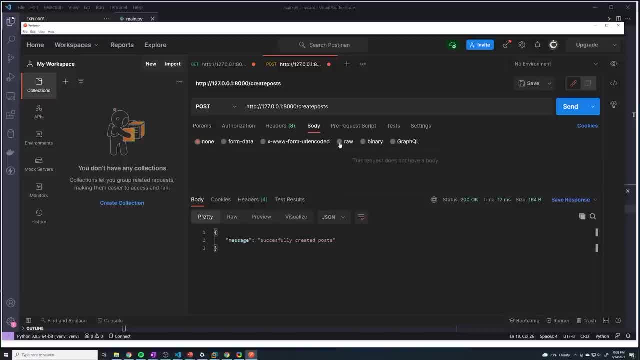 body section right here And then within body. what we want to do is go to raw and then select the type, And normally, when you're working with API's, you want to use JSON. However, you can use a XML and a few others. However, most people use JSON, So we'll select JSON. 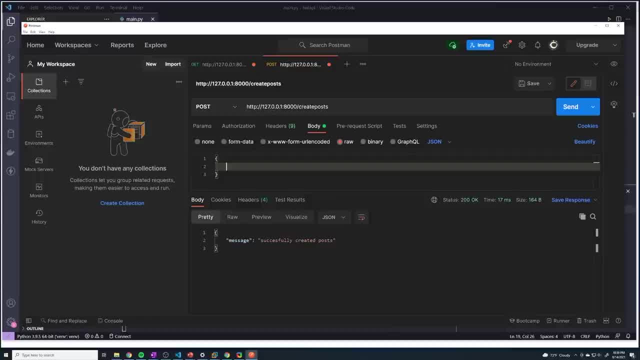 And then we'll do and JSON looks very, it operates very similarly to a Python dictionary. So it's, you know, curly braces and then it's going to be a whole bunch of key value pairs. So here I'll say what's the title of my post? Well, title my post is going to be say: I will say 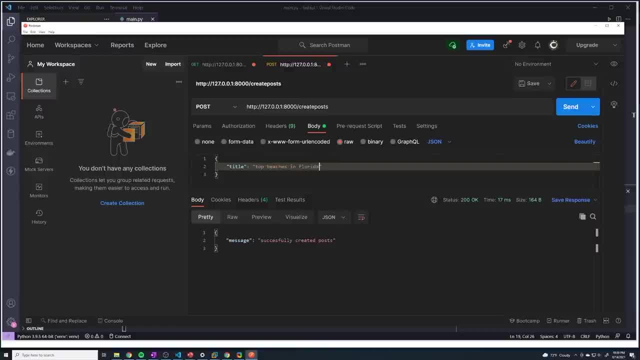 top beaches in Florida. And then the content of the post is going to say: check out these awesome beaches, Alright. and so now if we hit send, let's see what happens. Great. So it says: successfully create posts. we successfully hit this endpoint, But in our path, operation. 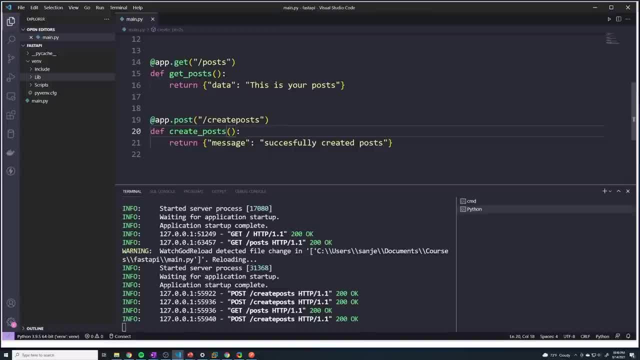 how do we actually extract the data that we sent in the body? How do we retrieve that body data? Well, what we can do is, within our path operation function, I can say I can just assign it some variable. So what variable do we want to store all that body data? you can pick any name you want. 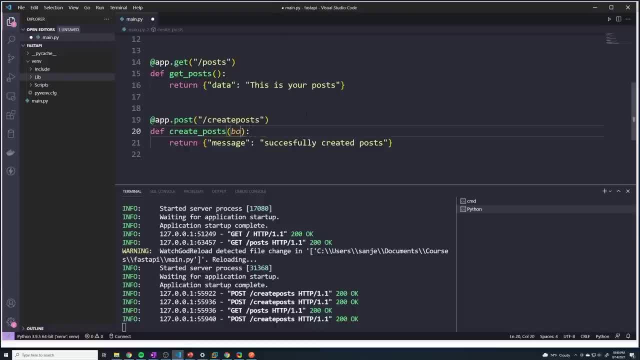 I'm just gonna say this represents payload, although it could be something like body or anything else. So we'll say payload, And then what we want to do is colon. And then we want to say it's going to be of a type dict And we want to set this equal to body And we want to import. 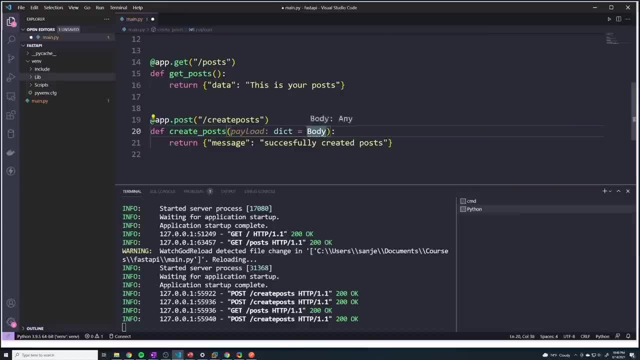 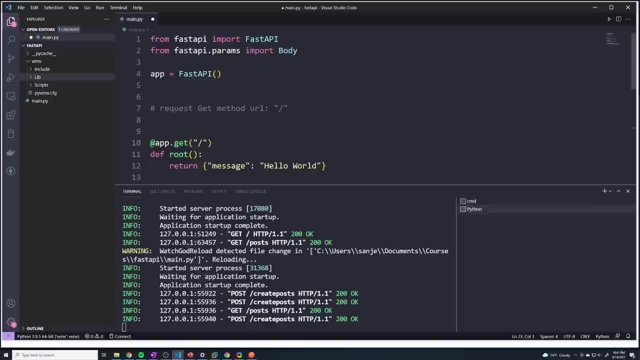 this. So this is actually something that comes from the fast API library. So if you do tab, if you hit tab, it's going to automatically import it or you can select it. So you hit body and then do that and then triple dots. And just to keep in mind, right, if you see that from fast, 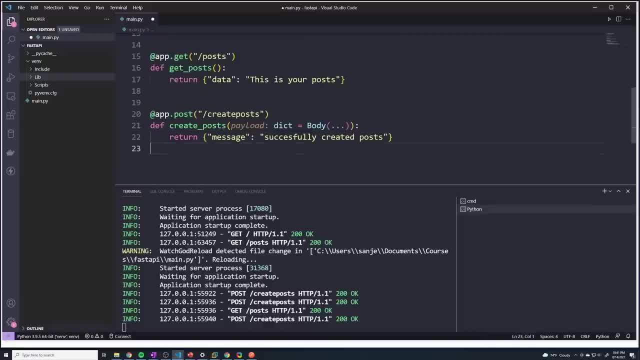 API params it imported body. So what this is going to do is it's going to extract all of the fields from the body, it's going to basically convert it to a Python dictionary And it's going to store it inside a variable named payload. Pretty simple And all we have to. 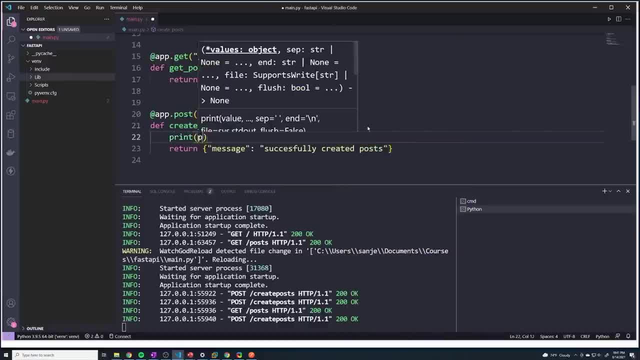 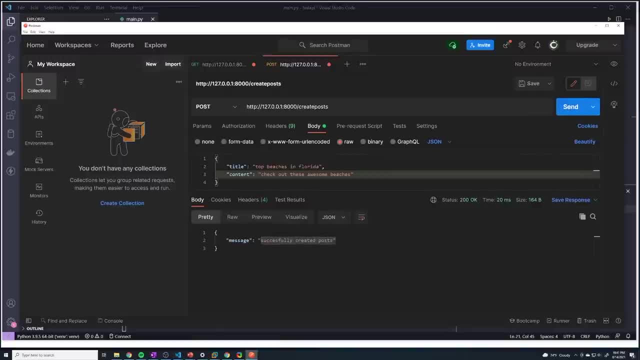 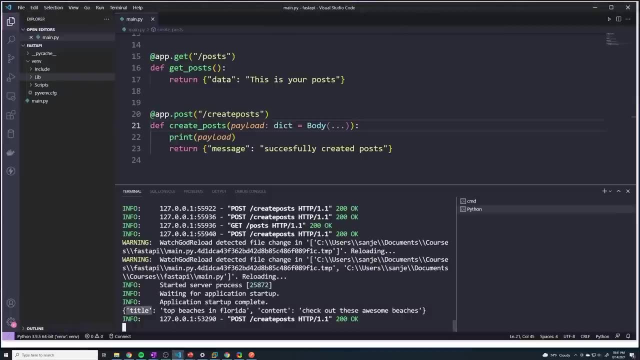 do is, let's say, print, Let's just print out payload. Now, if we hit that post request again, look at this right here- we can see that it converted into a Python dictionary and we extracted the title field as well as the content field, And so that's how we extract the. 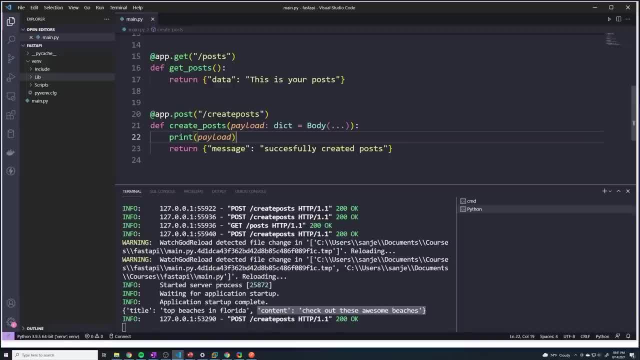 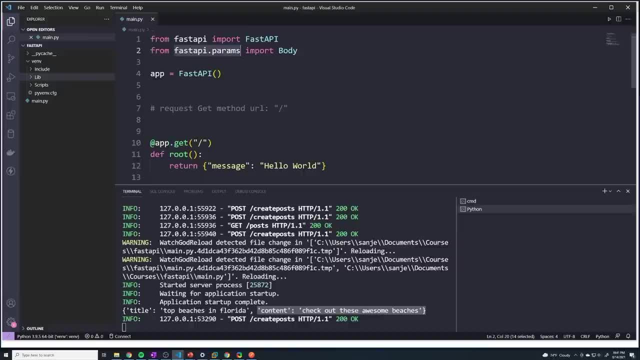 data from the body of the payload. All right, And just to quickly recap once again, we imported, we imported body from fast API dot params And we let VS code do it automatically for us. I always recommend letting VS code do it for you so that you don't have to memorize. 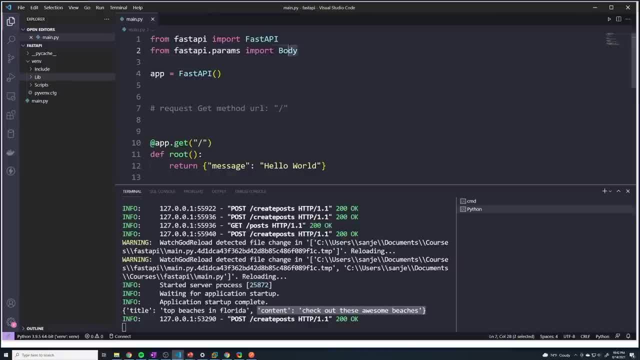 and remember you know where in the fast API library this, this property, stored. So we're taking this, taking the body, and then we're converting it into a dictionary And then we're storing it inside a property called payload. but you can name this whatever you want. 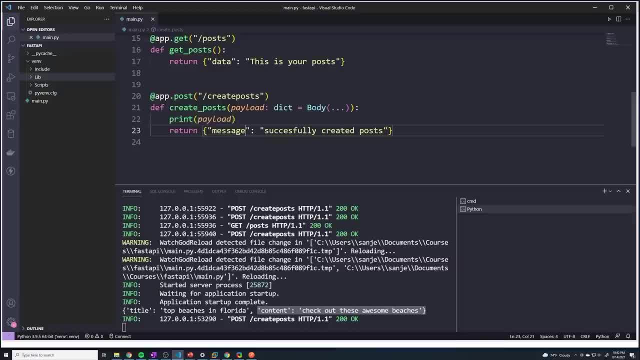 And so what we can do is we can take this data, and then we can, you know, we can take this data and we can say: let's say we're going to return back new, new post, and then we're just going to send the data. So we'll say: 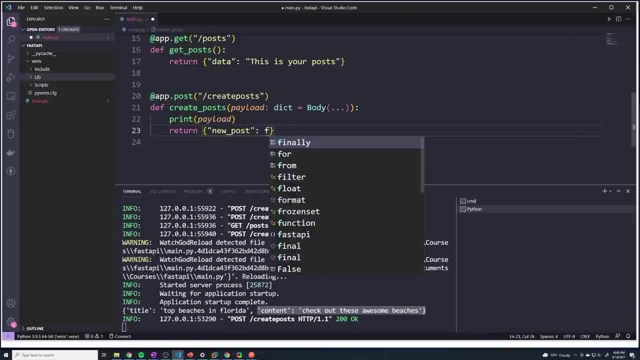 title And we can actually change this to a F string And we'll say title And then we can pass in payload And you'll see that we can just reference the title property, Because it's just a regular Python dictionary, And we'll say that the content is going to be: 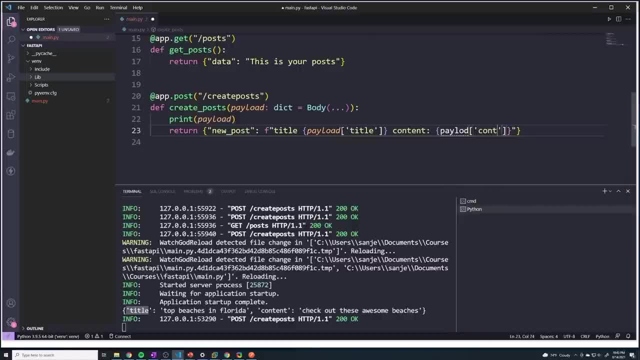 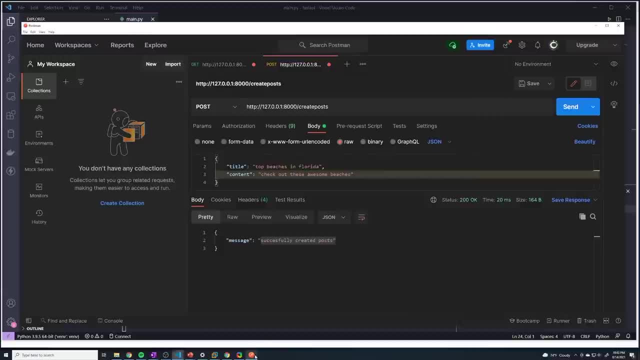 payload content. So let's save that, And then now let's hit Send. Now, look at this. we get our new post NSN. Whoops, it looks like I made a mistake. Yeah, no, actually, that's fine, We can change this, Okay. 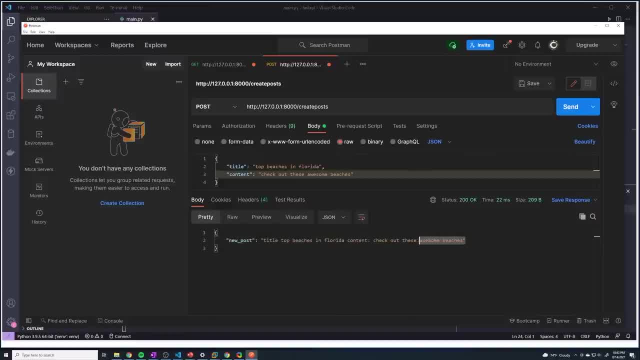 correct title of top beaches in Florida. content: check out these awesome beaches. So that's pretty simple, guys. I showed you guys how to not only send data in the body within a postman request. we're also able to extract that data and send it right back to the user. 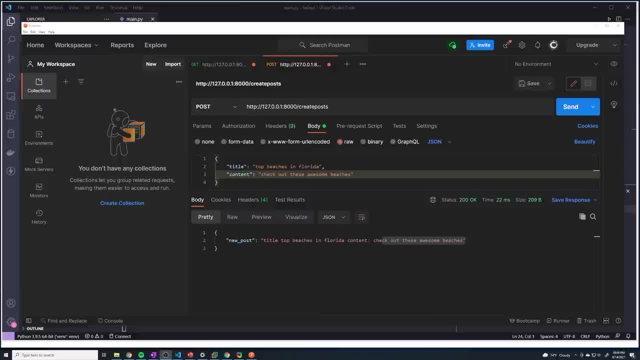 Now, in a real application, we would take the data and then we would normally store that data inside our database so that we can create a new post stored in the database And then now, anytime the user tries to retrieve the post, we can fetch that data from the database. 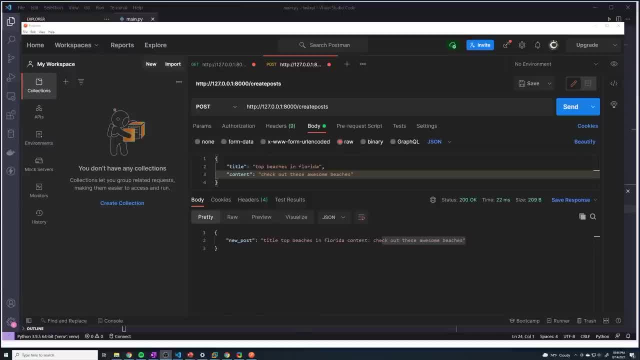 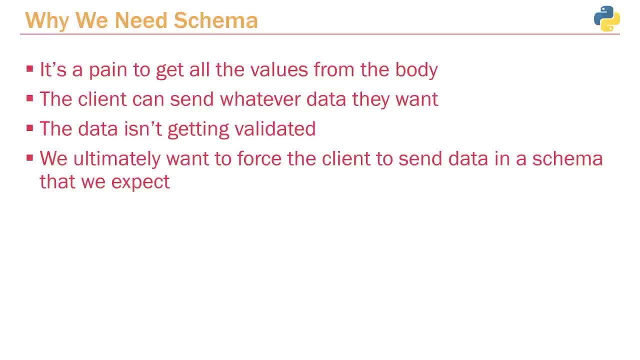 we don't have a database set up just yet, So for now I'm just showing you guys how to extract that data and then send it back in the request. In the last lecture we learned about how to work with post requests. we learned about 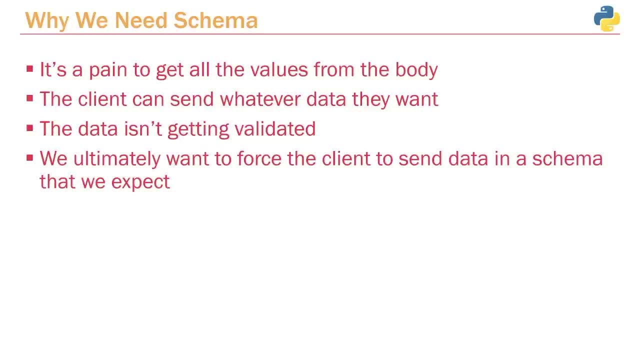 how to send data in the body using postman, as well as how to extract that data within our path operation, so that we can perform some logic, And there's some issues that we're running into at the moment based off of the way we've kind of set up things. 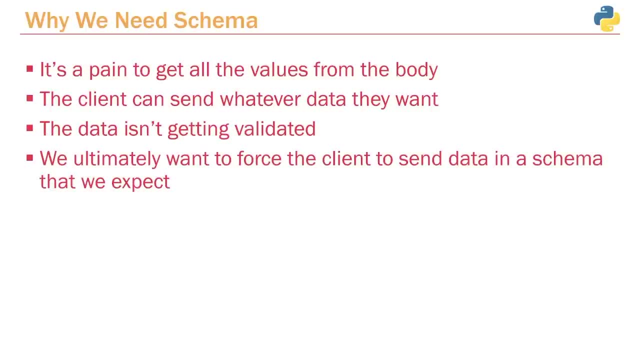 All right, and the first thing is it's kind of hard to get all of those values from the body. we have to, you know, extract each one individually. On top of that, the client can send whatever data that it wants. And this is a big issue, right? I don't want the front. 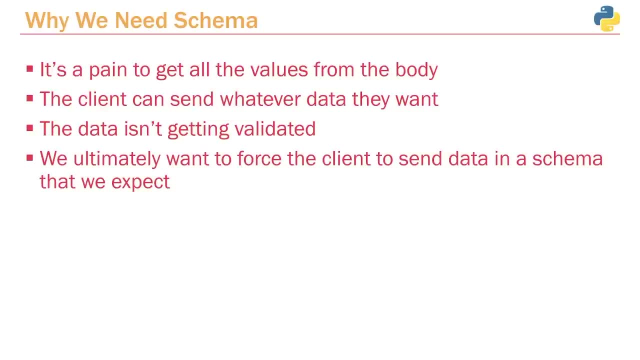 end to send arbitrary data. If the users trying to create a post- I want the title, I want the content, nothing else, Right? I don't want them to send any extra data And on top of that, the data itself isn't getting validated, Right? So how do I ensure that the user is? 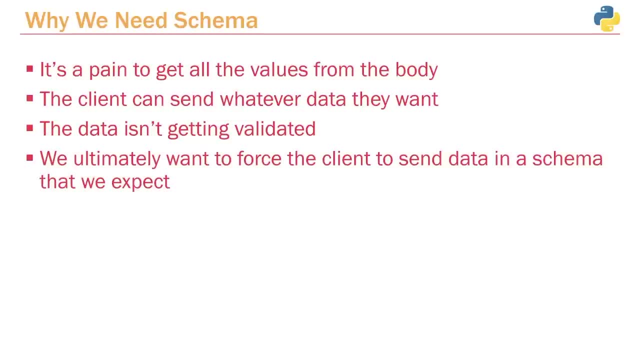 what I want, right. What if the user sends a blank title? I can't have a post with a blank title, So how can we validate that the data that the user sends is actually valid Right Now? ultimately, what we want to do is we want to force the user into a schema that we can expect. right, That's. 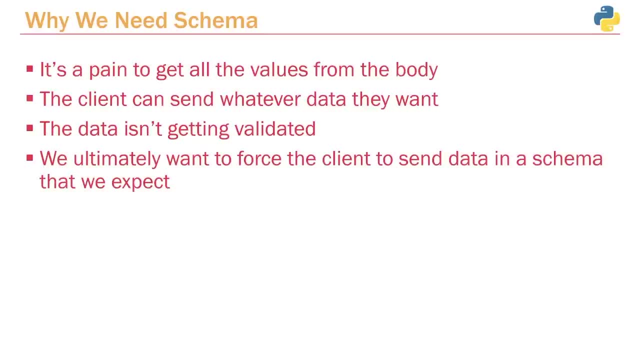 the term that we always use the API as a schema where we want to define exactly what the data should look like, so that it's almost like a contract between the front end and the back end saying, hey, the back end sends a message to the front end saying, listen, I expect my data to look. 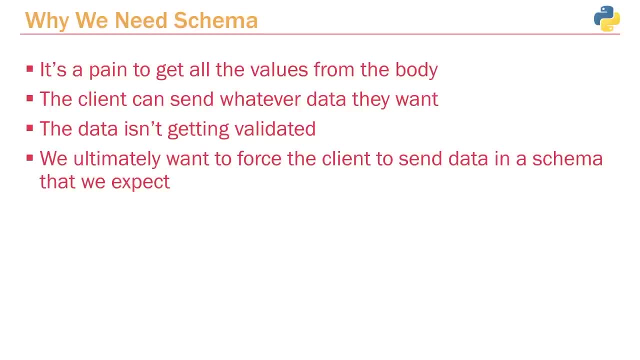 like this: If you don't send me the data that looks exactly like this, I'm going to give you an error, And that's the way you want to work with. API is you want to explicitly define what the data should look like so that the front end can send you exactly what you expected. So let's see how. 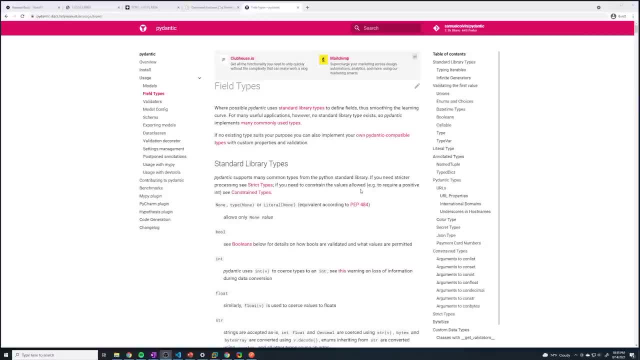 we can do that using fast API. Now what we're going to do is we're going to make use of a library called pydantic. Now we've already got this installed because we use that all flag when we did pip, install fast API. So if you actually go back to your code and go to your lib flag, 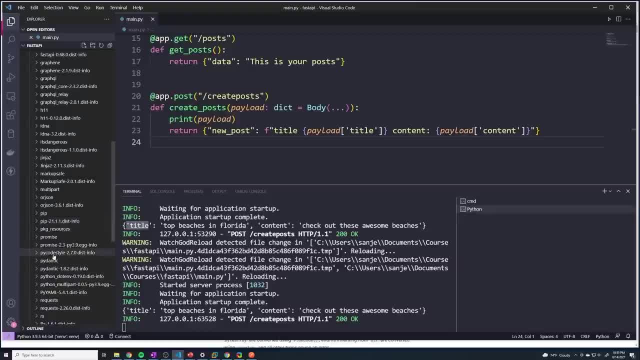 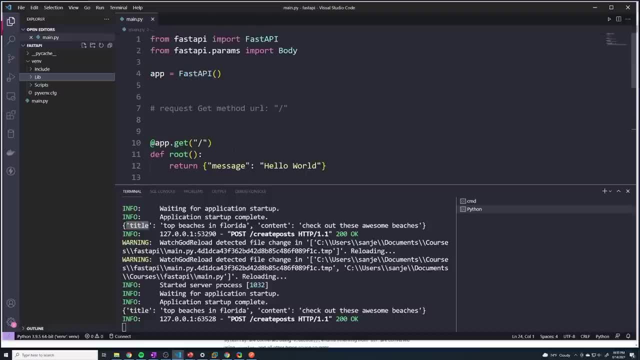 folder. you should see pydantic somewhere in here And you can see that pydantic is already installed, So we can make use of pydantic to define what our schema should look like. So let me quickly show you how to work with pydantic. It's really simple, But keep in mind, technically 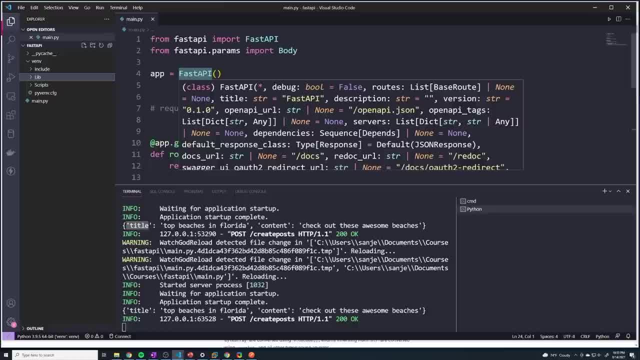 pydantic has nothing to do with fast API. It's its own complete and separate library that you can use with any of your Python applications. Fast API just makes use of it so that we can define a schema. So let's import pydantic. So we'll say from: 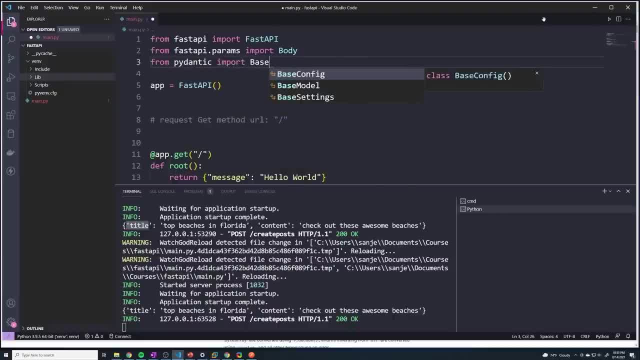 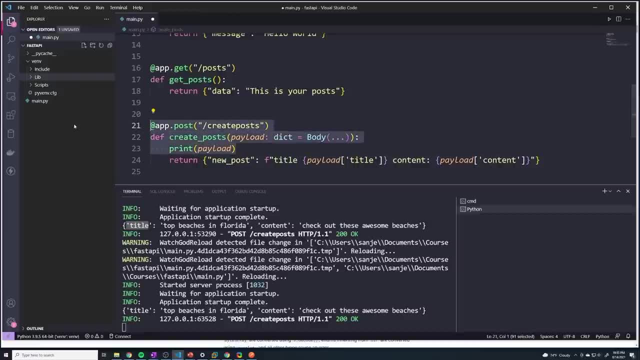 pydantic import base model. And so if we go down to our- you know our- create posts path operation, you know, ultimately, what we want to do is we want to tell the front end what a post or a new post should look like. what data do we expect? So let's figure out what data we want for 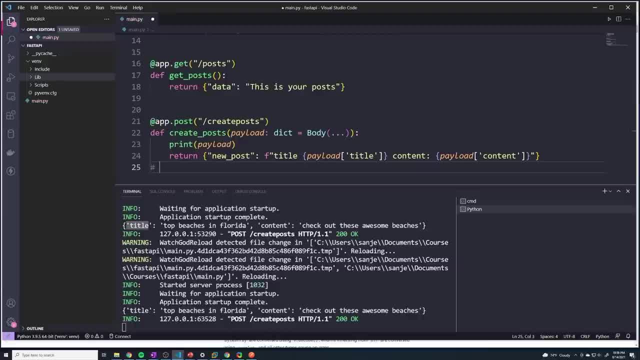 a specific post request. So two things that we want. we want a title which is going to have, which is going to be, you know, a string essentially, And then we want the content, which is the content of the post which is going to be. 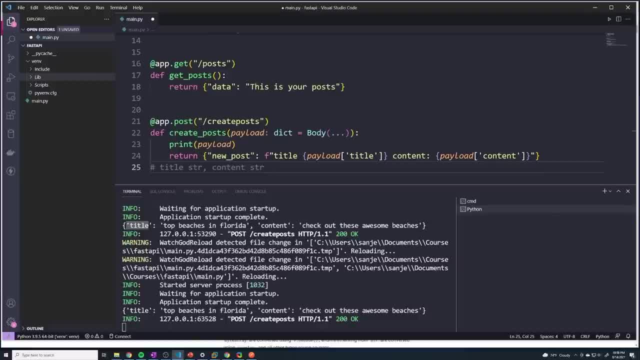 you know some sort of string Right, And so we want the. we expect the user to send both of those things, And then we don't really want anything else. We don't want the user to send any other piece of data, We just want these two things, And we can put in any other pieces of data we want. 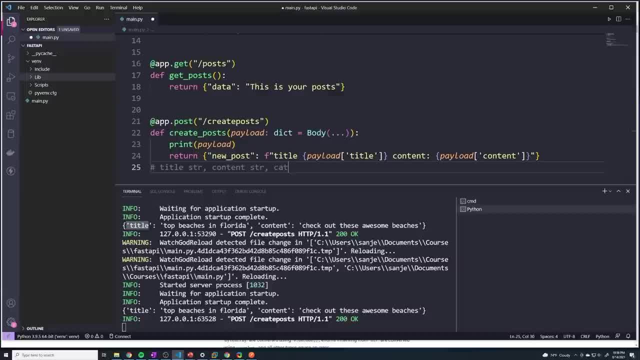 So if we want the user to pass in something like you know what is the category of the post, we can include that. We can maybe include maybe the number of- I mean, I don't know, you can really think of anything- maybe a Boolean that kind of represents, you know. 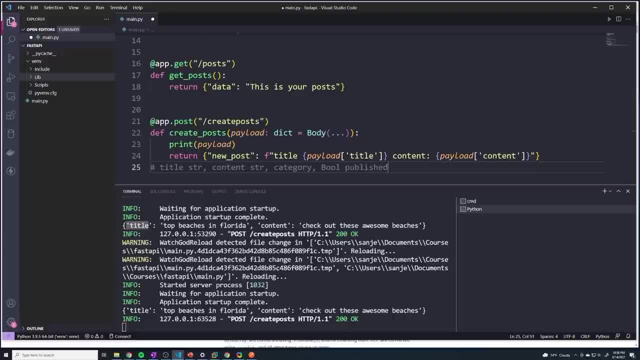 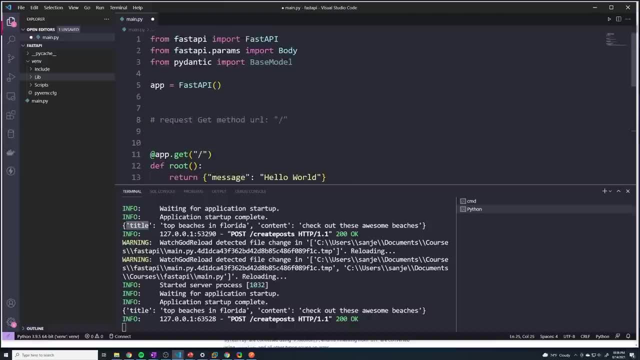 is this a published post Or do you want this to be saved as a draft So you can construct it however you want? But we're just going to stick to title and content. So the way that this works is I'm going to remove this comment right here. We're going to define a class. 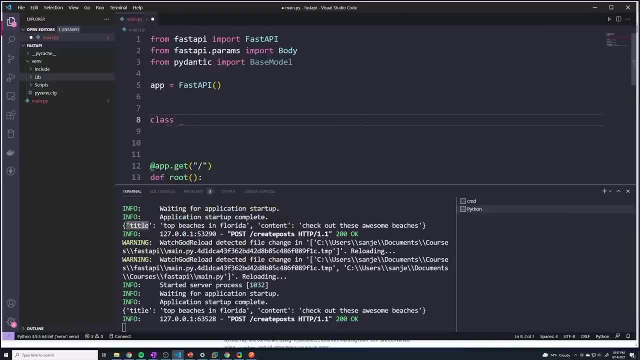 we'll call this class and then we'll give it whatever name we want. it's going to represent what a post should look like, So I'm just going to call this post And then this is going to extend base model. So this is what makes it a special pydantic model: we just extend the base. 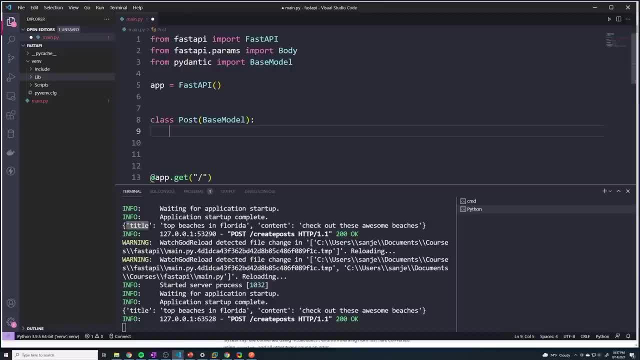 model And then here we pass in the different properties for our post And, like I said, we want a title And we also want a the content. Now, what we pass here is going to be what is this type of data? So if we go to this pydantic library, you'll see that there's the 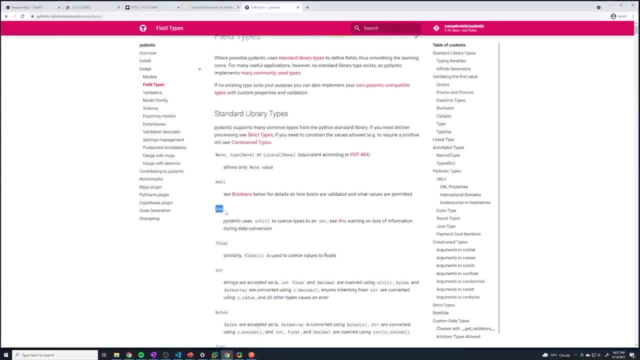 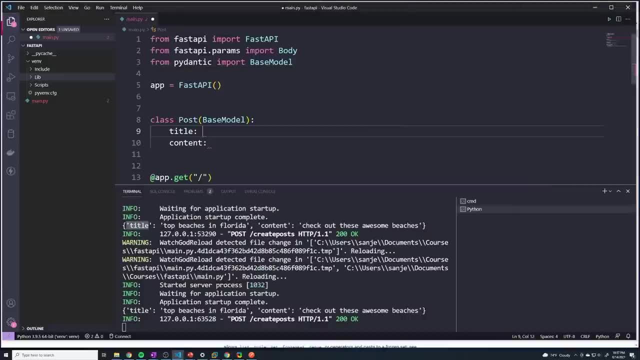 different field types. So we can set things to be a Boolean, we can set it to be an int float string, So all of the common Python types list tuple. it's all available within pydantic. So we know what a, ultimately, what a title should look like. So what do you guys think? 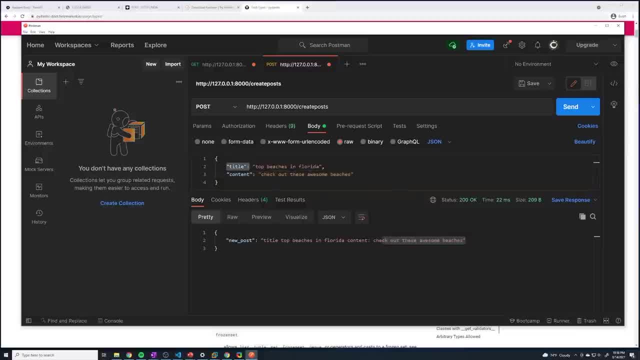 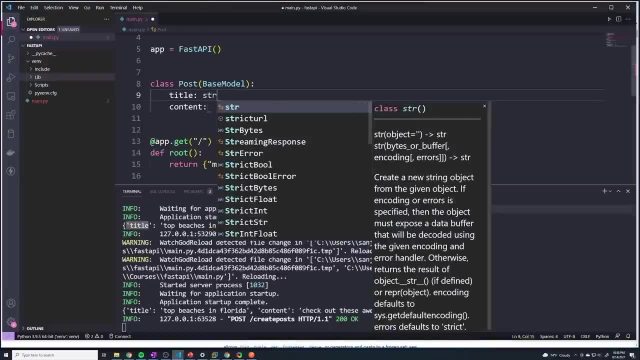 should be the field type for the title property. Well, I think it makes sense. is it should be a string? because this looks like a string. It's got some text. it probably should be a string. So let's set this to be string And the content should be the same thing. It should also be. 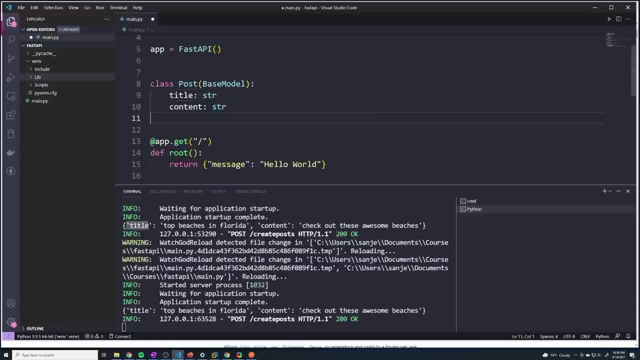 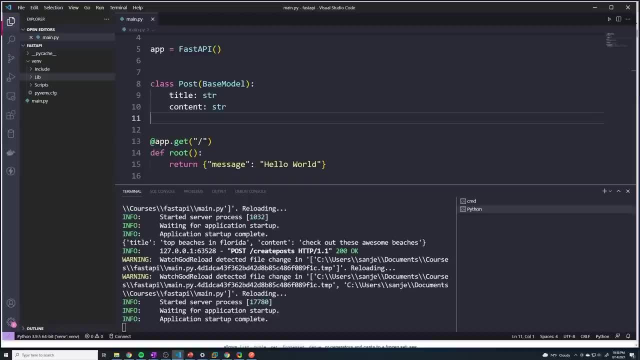 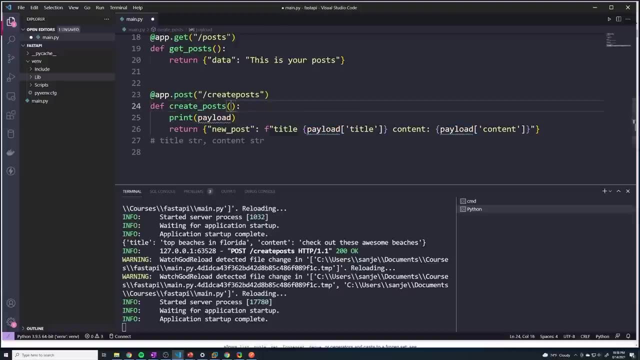 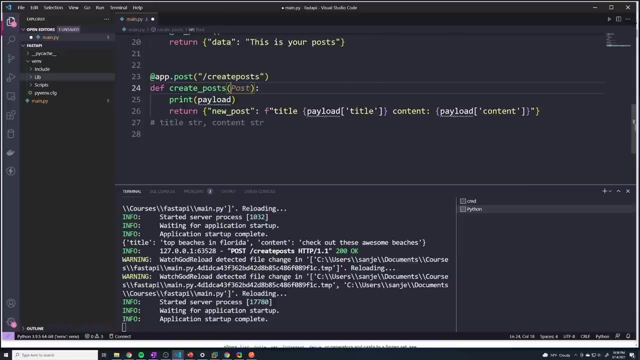 to string. And now what we can do is: let's take this model and go down to create posts Instead of extracting the payload. what I'm going to do is I'm going to reference that post pydantic model And then I'm going to save this as a variable called post. Once again, they don't have to match. 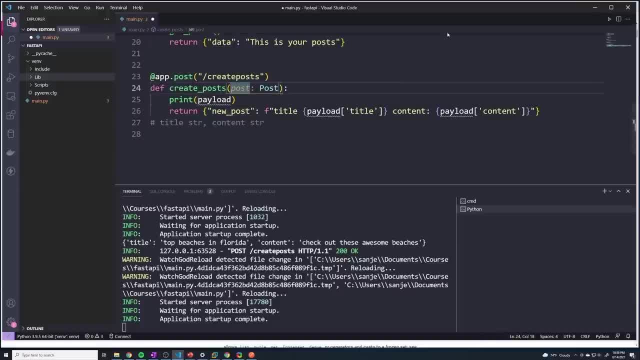 But since this will represent the post, I can call this maybe new underscore post or something like that, And then and then reference the post: pydantic model. So what's going to happen is, because we pass this into our path, operation fast, API is automatically going to validate the data. 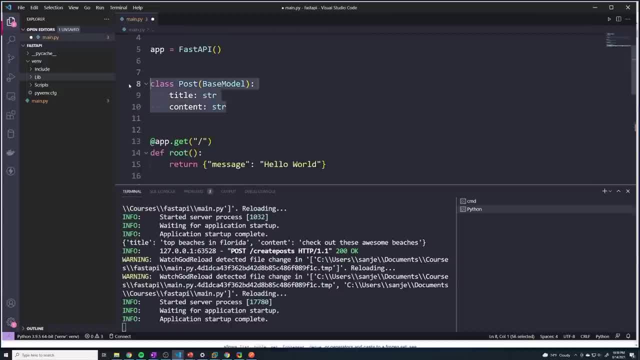 that it receives from the client based off of this model. So it's going to check. hey, does it have a title? If so, is it a string? If it, if the title doesn't exist, or if it's not a string, and maybe 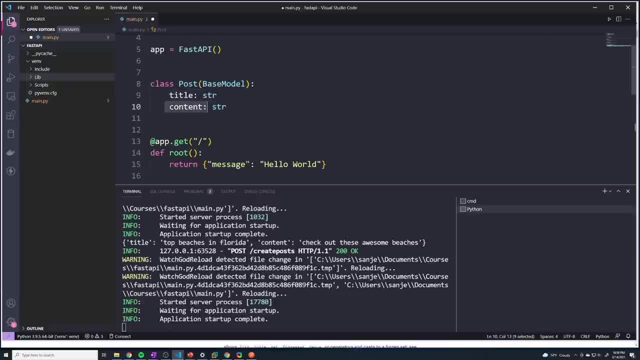 we pass an integer, then it's going to be a string. And then it's going to check: hey, does it have a title? If so, is it a string? And then it's going to throw an error. it's also going to check for us. 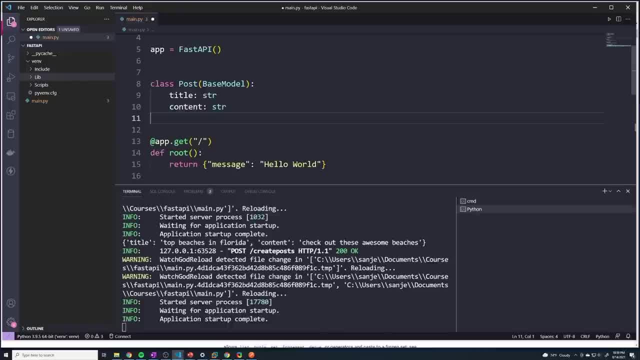 if contents available. If it is available, it's going to make sure that it's a string, And if contents not available, or if it's not a string, it's going to throw an error. So it's doing all of the validation for us And it's defining the scheme of what it should look like for the front. 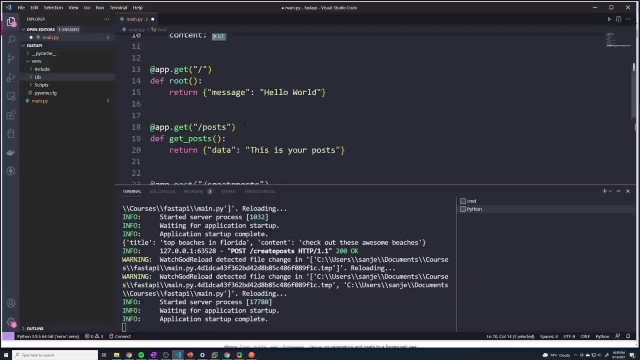 end. What kind of data should the front end send to us? So we're going to remove all of this nonsense. I'm just going to, for now, just say data, I don't know, new post for now. And now I'm going to do: instead of print payload, we're going to say: 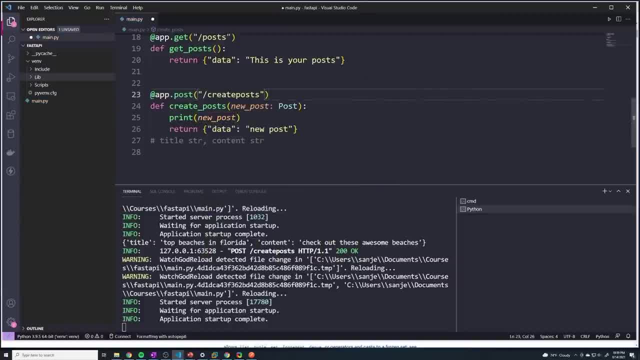 print new underscore post. So let's save this And then I'm going to send a post request. Okay, so that update is fine, But let's take a look at what this printed out. So take a look at what I printed out. look at that. it automatically extracted all of that data for us, So now we can access in a post. 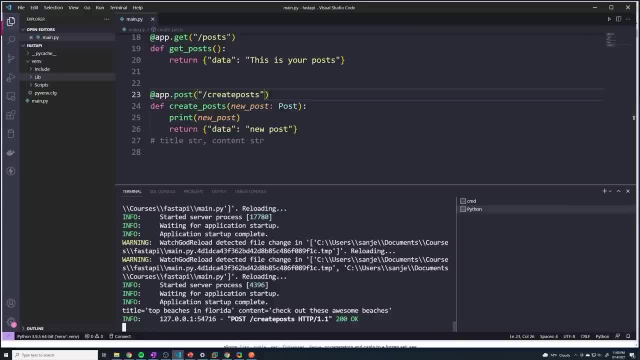 dot title And we can get the title of the post And we can also access post out content to get the content of the post. And just to prove that to you guys, we'll say post dot title. So we'll save that. we'll send a. 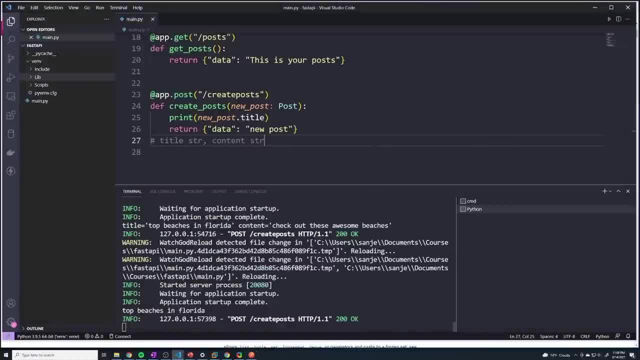 request And now look at that. look how easy it is to extract that data, because it's already assigned to that new post variable And we can just access each property based off of what the model is defined as. Now that's great and all, But let's check to see if it's. 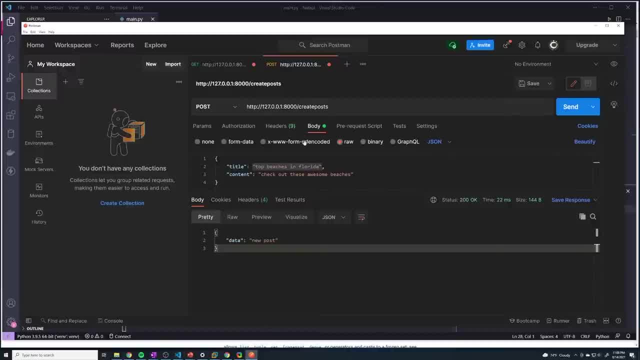 actually performing all of that validation. So if I go to my postman and I remove title- let's see what happens- I'll hit send. Look at this. look at this. it's saying that the inside the body, there's a. 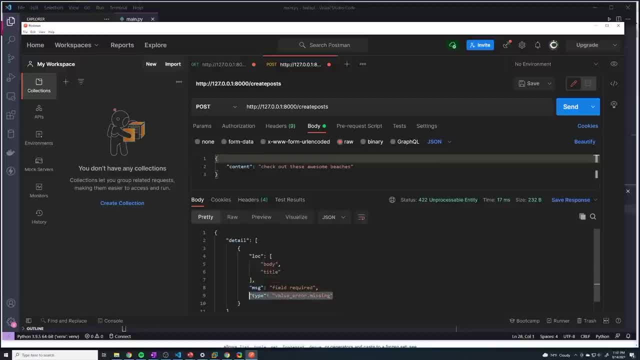 title field and it's saying a value error. it's missing. Now we didn't tell fast API to send this, but it automatically does the validation for us and sends back an error message And then it sends back a status Code. So this is the status code of the message. it sends a 422.. We can change that later, don't worry. 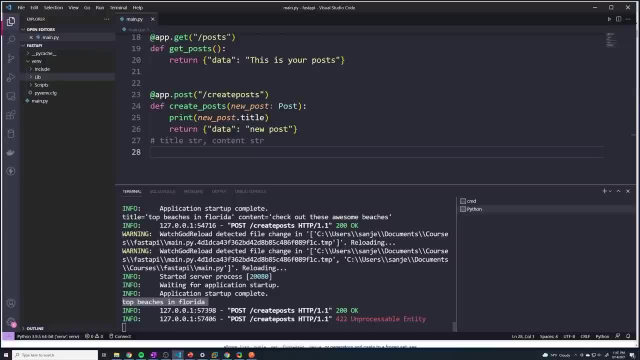 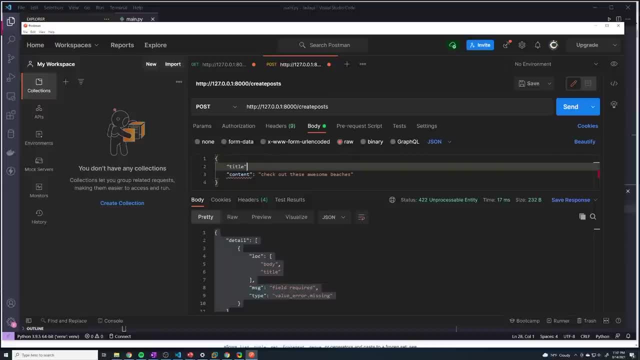 about that, But it's automatically performing the validation And that's what's awesome about this. And if we, if I add the title back, what was it? top beaches in Florida, And instead actually I changed this to be a one or something, And I need that comma. Let's see what happens if I hit send. 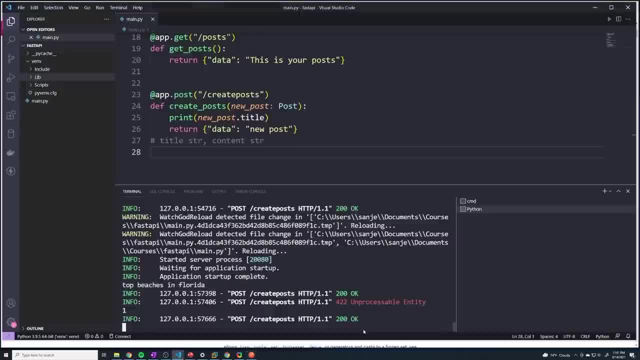 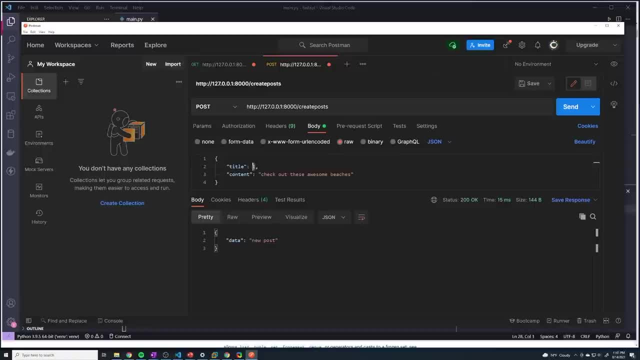 And that's because the number one can actually be converted into a string. So it's not going to throw an error on that, And that's perfectly fine, And I'll, and that's perfectly fine. So that's not a big deal. But let's change this. 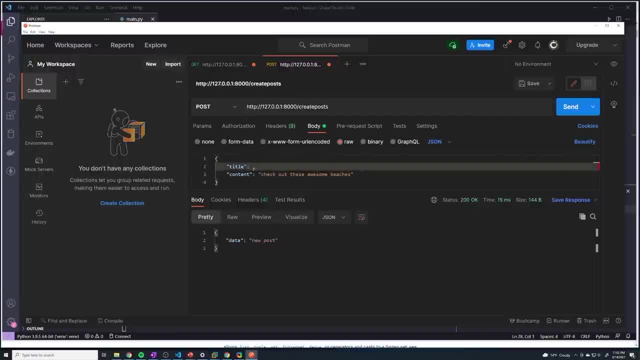 back. Like I said, it's going to try to convert whatever data we give it to a string. So as long as it's able to convert it to a string, it's okay, And any integer that we pass can be converted to a string. So I'm going to change. 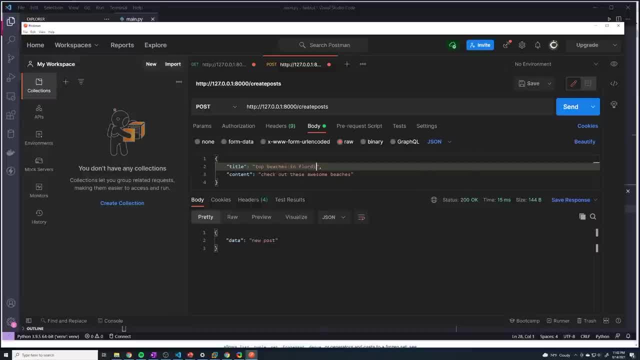 this back and I'll add top beaches And Florida, Florida. let's see what happens if we remove the content. now I hit send. Look at that. Now it's saying the content is missing. Perfect, So our validation is working exactly how we expect it to. And then I forget what. 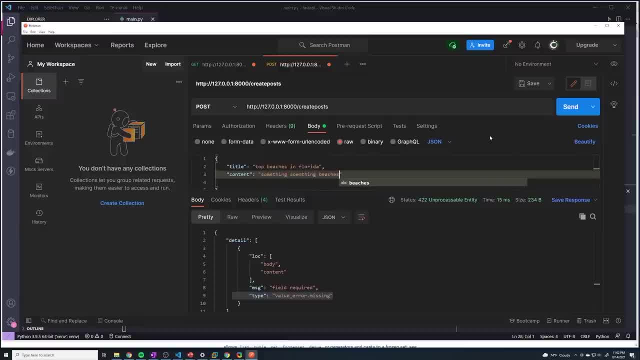 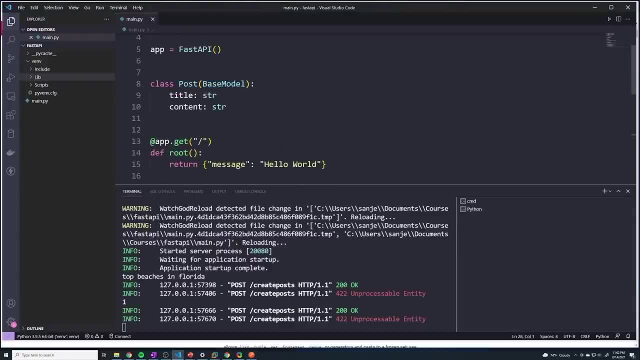 was it? Something, something, beaches. I can't remember what it was. Now, let's say that we want to assign a property that's optional right, Like what? if we want it to make it so that the front end can either choose: 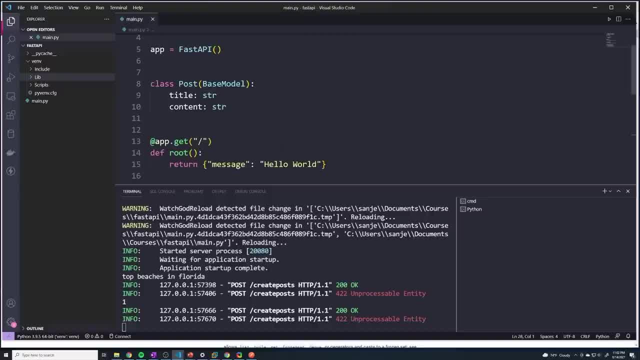 to send some piece of data or not send a piece of data. So let's say that we want the user to be able to define if a property, if a post, should be published or not. well, we can create a field called published, which is going to be set. 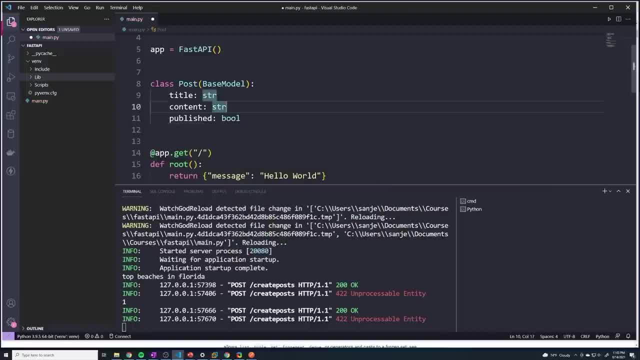 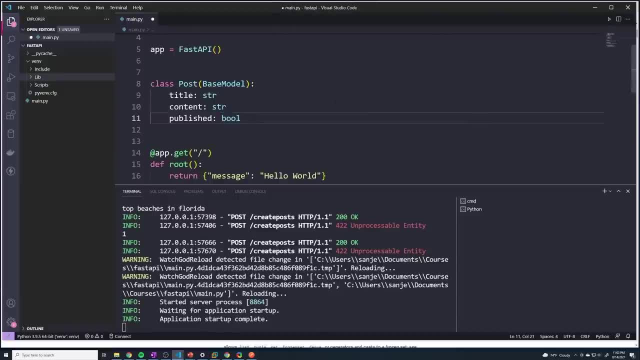 which is gonna be a type of Boolean, And we can say: you know, first of all we can say: if the user doesn't provide us a value, we can give it a default value. So here I'll say true. And so if the user doesn't provide published, then it's going to default to true. If it does provide published, then whatever value you give it, that's what we're going to use it as, And I'm going to go down here And we're going to change this to: we're going to grab the published value. 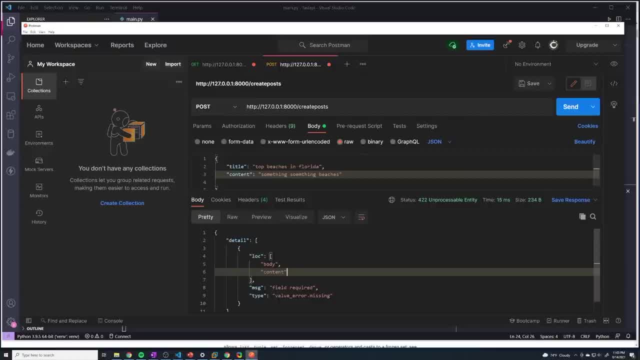 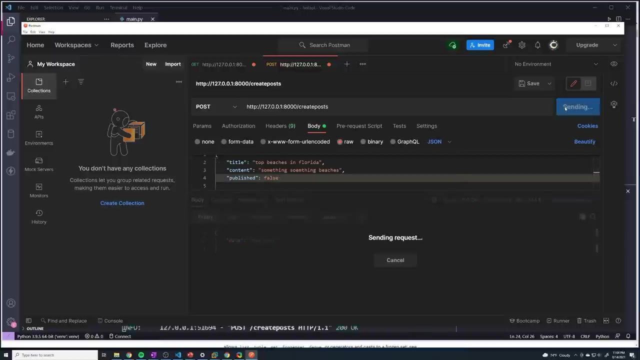 And then down here we'll say: published whoops can be set to true. So let's hit send And we can see that it got set to true. that's good. If we set this to false, it send. we can see that it's false. And then if we remove this altogether, 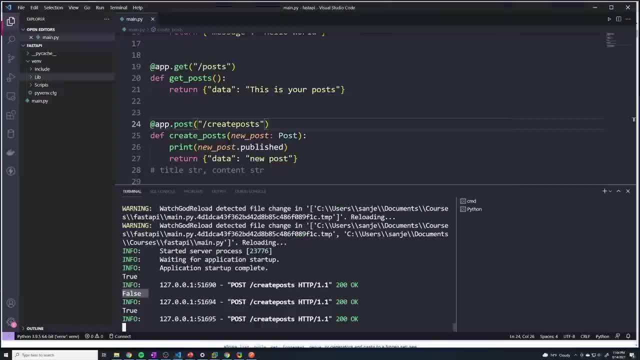 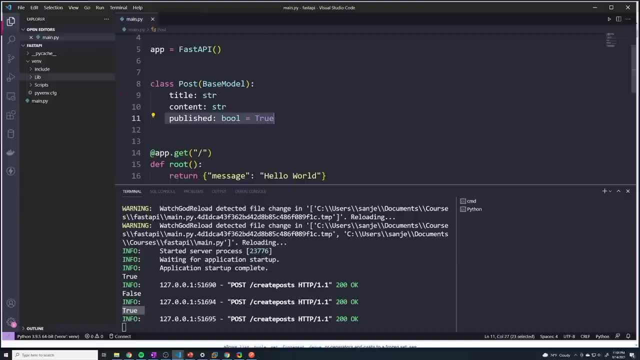 move that comma as well. Hit send. Look at that. it defaults to true. So now we've created an app, an optional field for our schema, So the user doesn't have to provide this and it's going to default to true in this case. 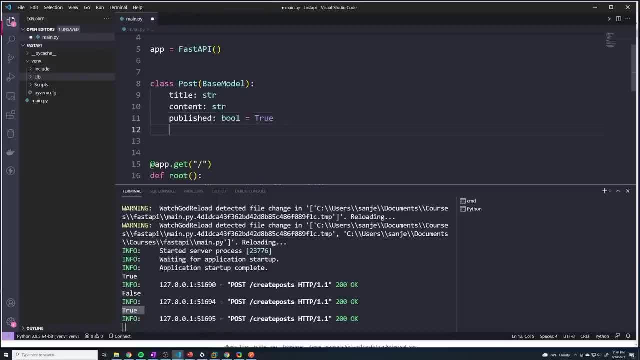 Now, let's say we wanted to create another field. However, instead of giving it a default value if it's not sent, we want it to default to none. So we want it to be completely optional And we're not going to store any value. 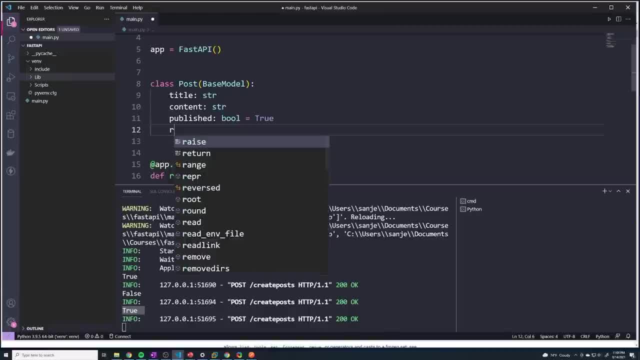 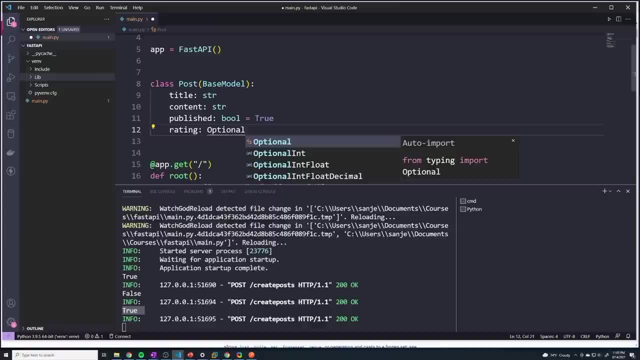 If the user doesn't want to provide it. what we can do is, let's say the field is a rating. let's say the user can give each post a rating. what we can say is optional And we're going to have to import optional from typing from. 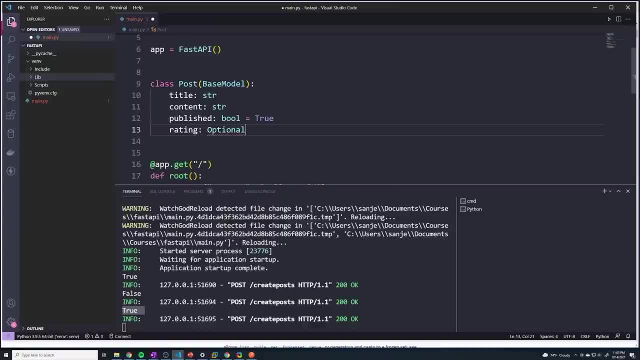 the typing library. So import optional, And then we have to pass in the type. So what is going to be in this case? a rating? I think an integer makes sense, And then we can say: equals to none. So this is going to be a fully optional field, And if the user doesn't provide it, 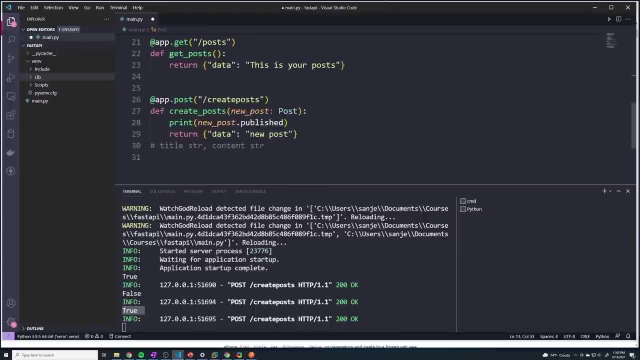 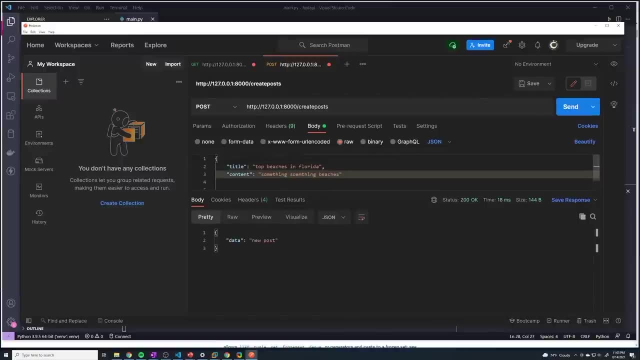 it's going to default to a value of none. And so here I'm just going to get the, the value of our rating. And so if I hit send right now in our body we don't have a rating field- I hit send, you can see that it defaults to a value of none because we set this to be. 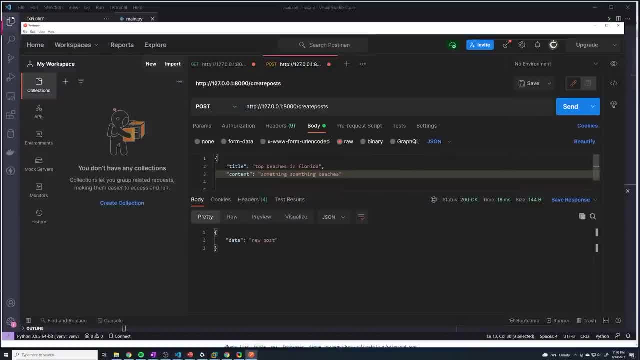 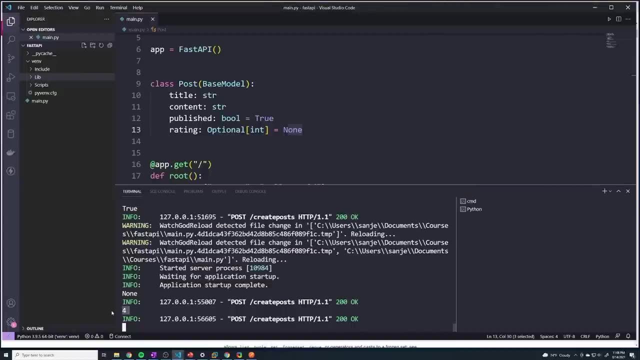 optional, none. However, if I pass in a rating field, I need to get it a value, some kind of value. So I'll say we'll give this maybe like four stars or something. I hit send. we can see that now. look, the value of rating is set to four. 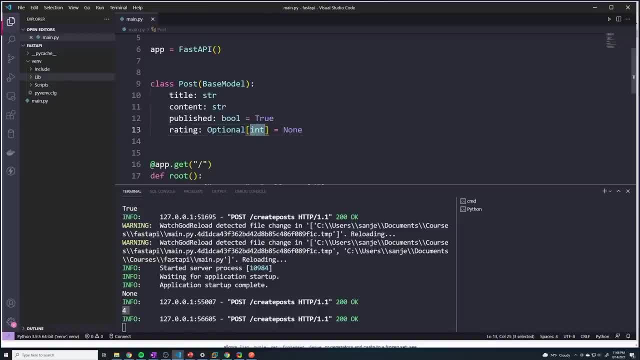 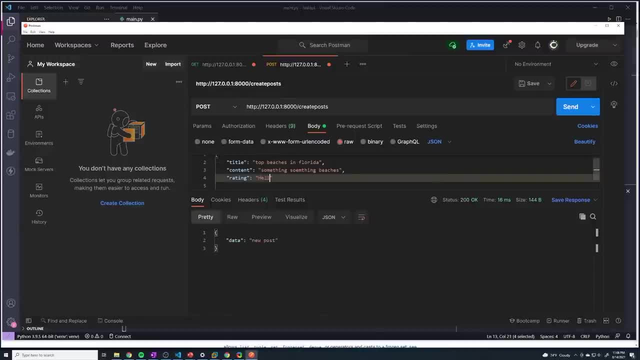 And then, finally, the last thing I want to note is because we set the type to be an integer. So even though it's optional, we still have to specify the type. If I give this a value of a string, so you know, something like hello, which is not a valid rating. 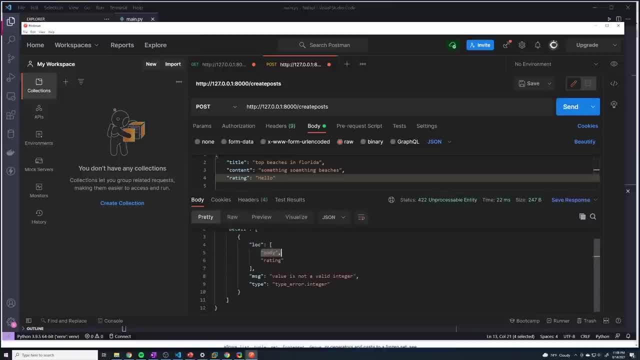 take a look at what happens. Look at that. It says in the body: the rating field, the value, is not a valid integer. So it wasn't able to convert whatever value we sent into integer, And so that's why it's throwing in and saying like: this does not. 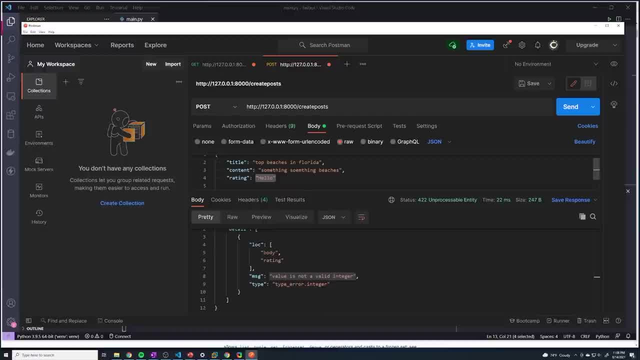 match up with schema and it's throwing an error, And so that's what's awesome about this is now we can ensure that our front end is sending the exact data that we expect by using these pydantic models. So, moving forward in this course, we are going to really make use of. 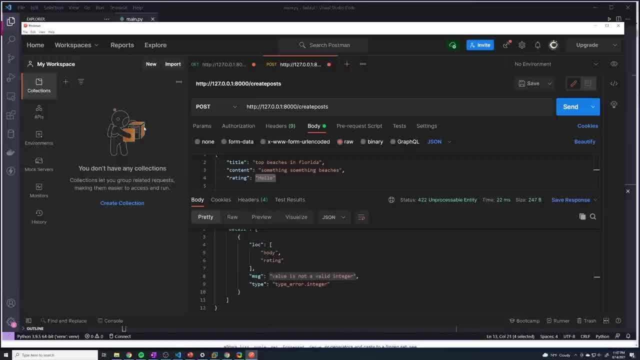 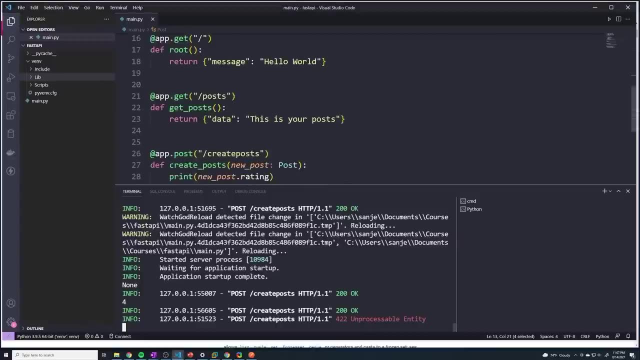 pydantic models to ensure that the schemas not only receiving data from the front end but also sending data back, is all matching up with our organized schema. And actually there's one last thing I want to show you guys, And that is that when we actually kind of extract that data and 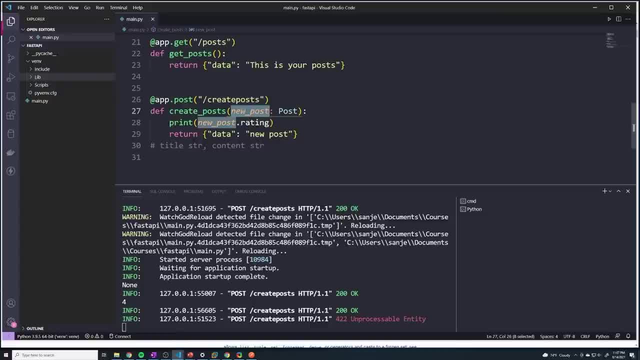 save it into new post, it actually stores it as a pydantic model. So it's a specific pydantic model And each pydantic model has a method called dot dict. So if I do, if I print new post below this: 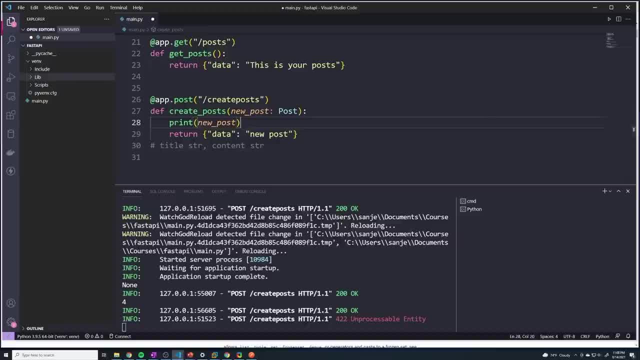 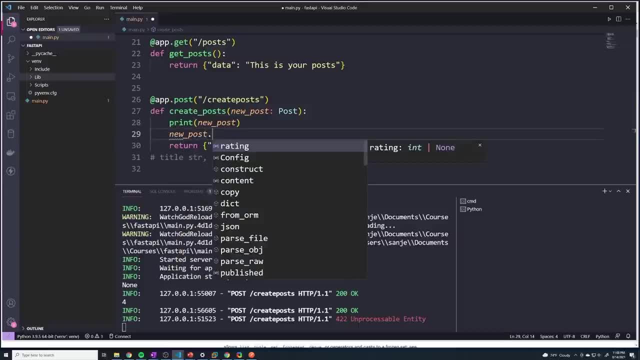 what we can do is, if you ever need to convert your pydantic model to a dictionary, all we have to do is write the name of the variable and we say dot, dict. This is going to take that pydantic model and then it's going to convert it to a dictionary, So let's print that out. 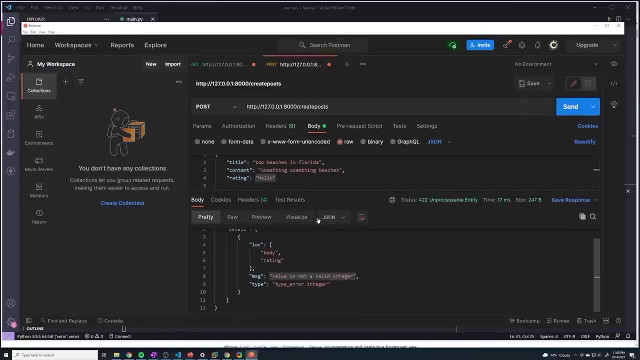 Let's save it, Let's hit send website, And I forgot to. it's still throwing a validation error, but that's to be expected, So we'll say: change that to four. I take a look at the two different things. So this is a pydantic model. 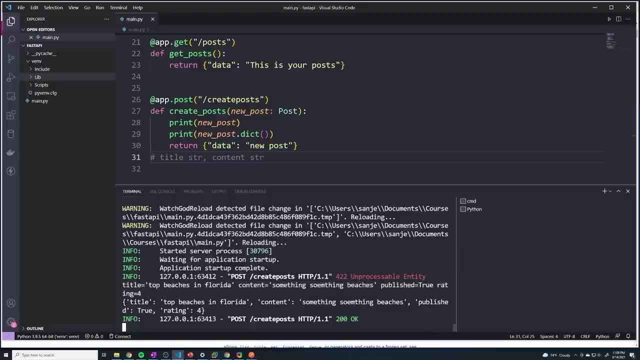 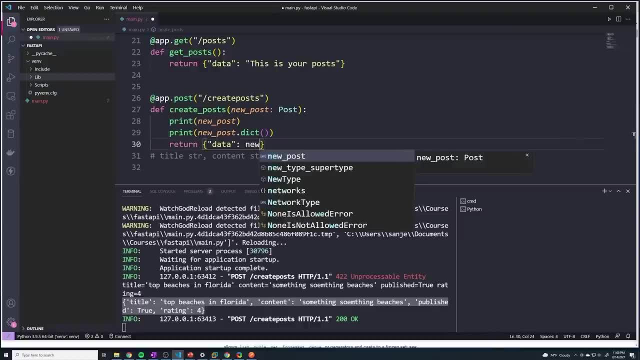 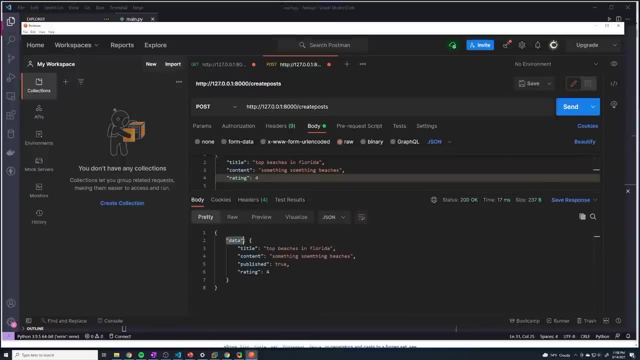 that's just printing out the different properties of that, of that model, whereas this is a regular Python dictionary. So we can just send back a dictionary if we want to. So we do return new post and save that. now, if I hit send, we're just sending back a dictionary, And so now we send. 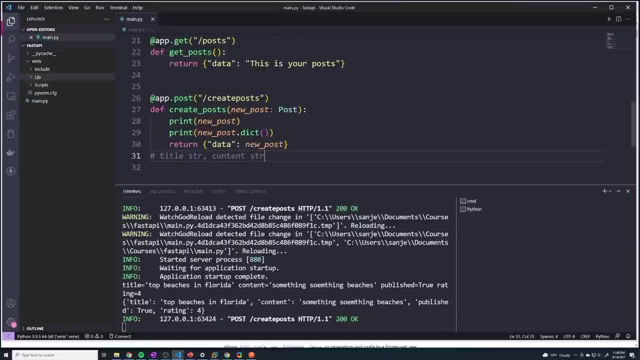 back the data with all of the different properties, And so you'll see that this is actually a nice little handy tool to be able to convert it to a dictionary, which is something that we'll be needing to do in some of the future lectures. 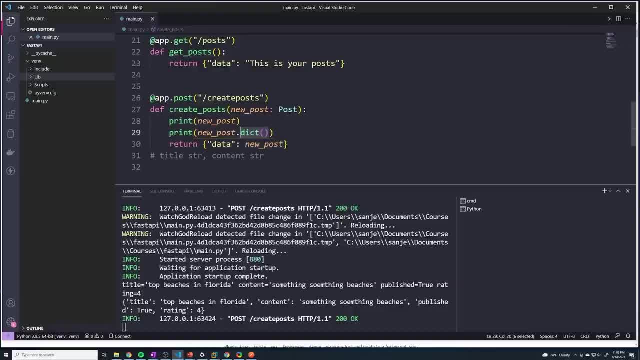 So I wanted to make sure we just cover our bases real quick on that And also I don't like calling this new post. I'm just going to change this to post for now, because I think that's a little bit better my opinion, because it is just a post. we don't need to know that it's. 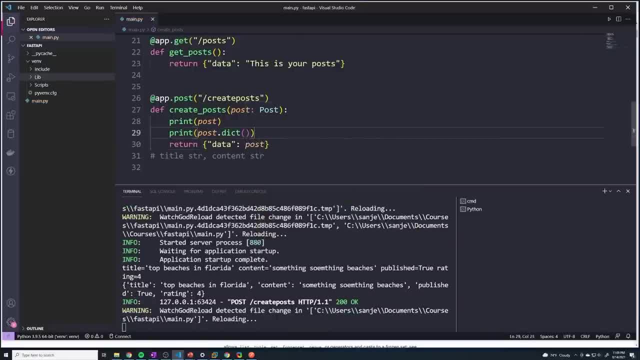 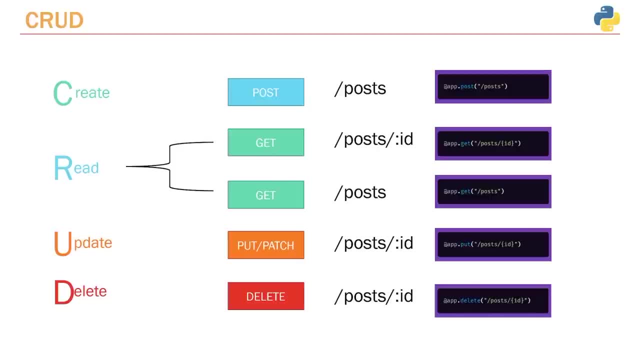 a new post. it clearly is, And let's just double check that everything works. Hit send Perfect. In this lesson, we're going to talk about what a CRUD application is, as well as what our standard conventions when it comes to creating an API for a CRUD based. 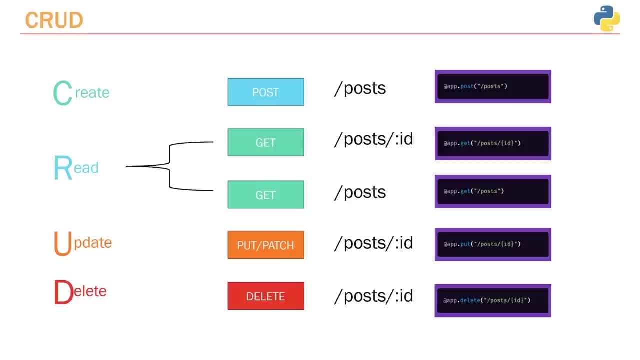 application. So CRUD is an acronym that represents the four main functions of an application. So any application, regardless of what it is, needs to be able to create things. So in our case, since we're building a, you know, a social media type application, 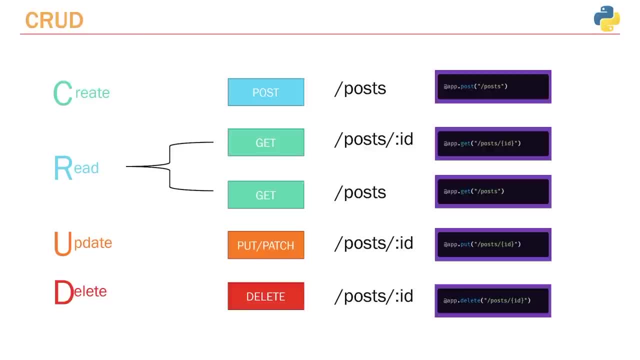 we need to be able to create posts, make new posts, we need to be able to read posts, And so that includes, you know, retrieving all of the pre existing posts. we need to be able to update a post if we want to implement that functionality, So if we decide to change what our post says, 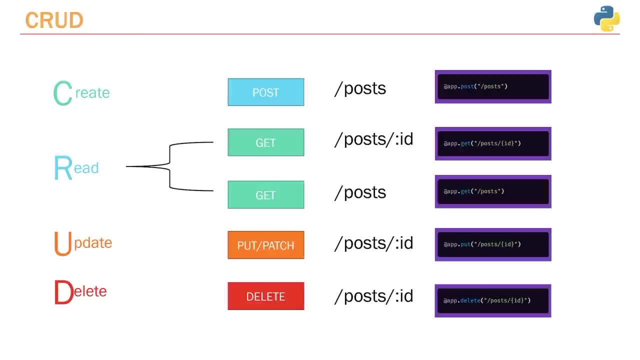 we would use the update functionality, And then, finally, we need to be able to delete a post, And so the CRUD- that represents the four main functions of any CRUD based application. so it's nothing more than an acronym. However, I created the slide so that you guys can understand. 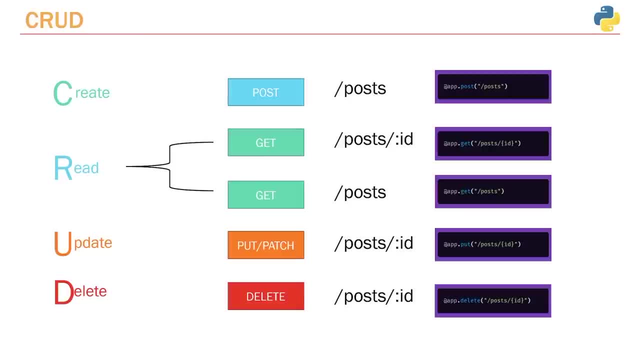 what our standard conventions when it comes to creating an API for a CRUD based application, because there are certain best practices and best practices that you can do to create a CRUD based application. So when I started in the past, I think I was in the business of creating an API. 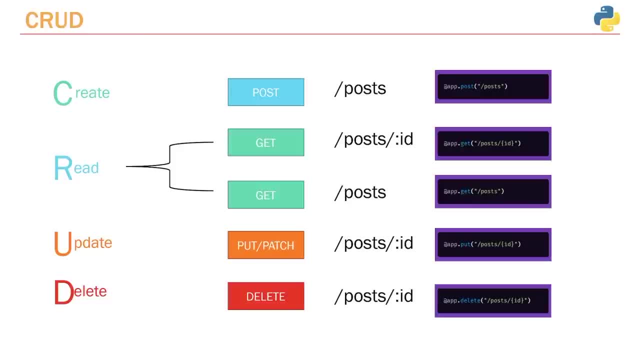 best practices that we need to follow, And so, when it comes to naming the URL and the paths for each operation, there's a standard convention, And the first thing that I want to point out is, since we're working with posts, it makes sense to name all of the URLs, all the paths, with slash. 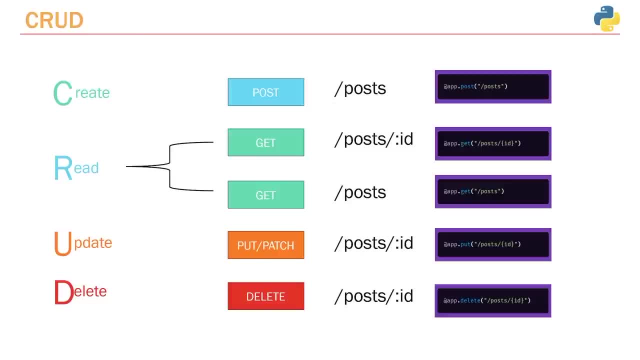 posts And it's important that you use the plural form of posts. You don't want to do slash post, You want to do slash posts as in plural. This is standard convention for APIs And if we were working with users and we want to do be able to create, read, update and delete users, it wouldn't 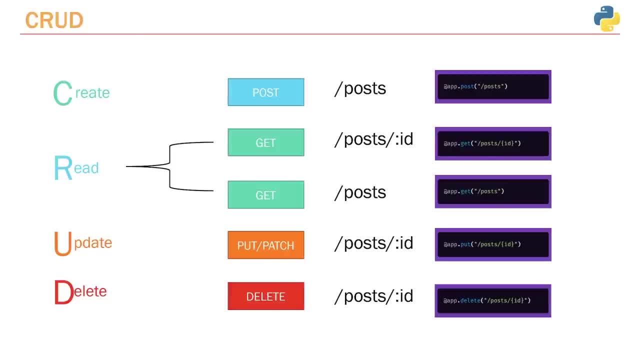 be slash user. it would be slash users, So always use the plural that standard convention. Now, when it comes to creating a post, right, that's always going to be a post request. So we've got the create functionality right here And we can see that we have to send a post request standard convention. 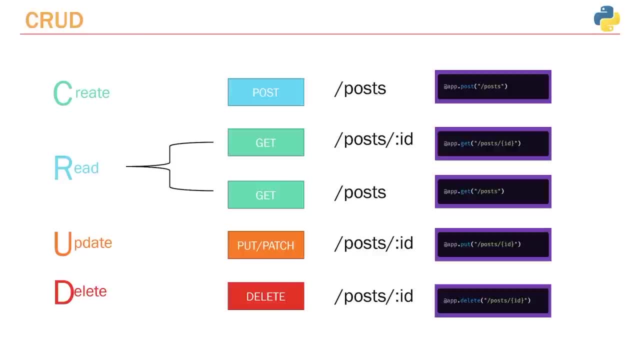 anytime you want to create an entity, it's going to be a post request And the URL or the path for that specific request is always going to be slash Post in this case, And if you want to see what that looks like for the decorator and fast API. 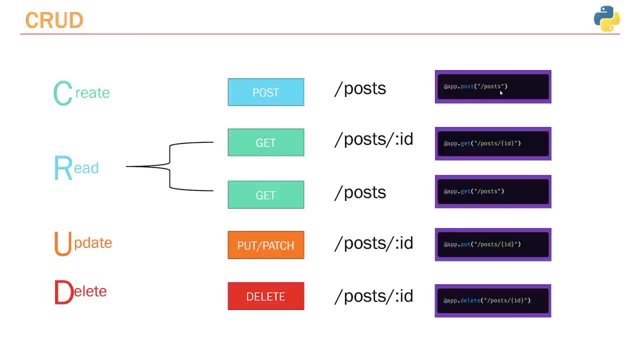 it's pretty simple. you just do app, dot, post, slash post. So this is something you guys already know. Now, when it comes to read functionality, which would be, you know, reading or retrieving pre existing posts, there's actually two different path operations we're going to create. 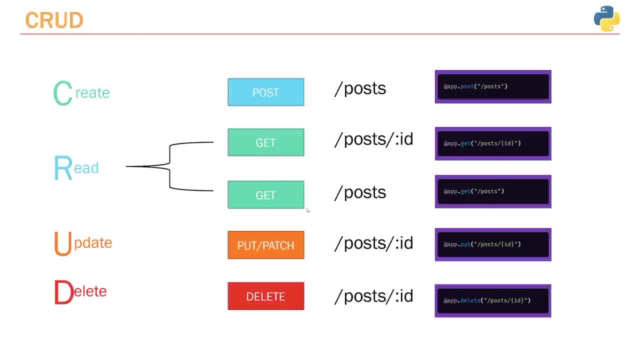 So the first one is going to be slash posts, And this is going to be for retrieving either all of the posts or multiple posts, depending on what filter that we use. And so when it comes to retrieving information from a database or anything like that retrieving data, it's always going to be a get operation, So you send. 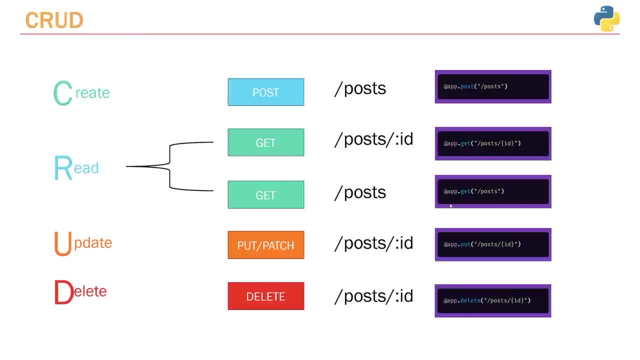 a get request to slash posts And if you want to see what that face the decorator on fast API would look like, it's just app dot get slash posts. Once again, we already have this set up in our application so far. However, there's also going to be another path operation for reading right. 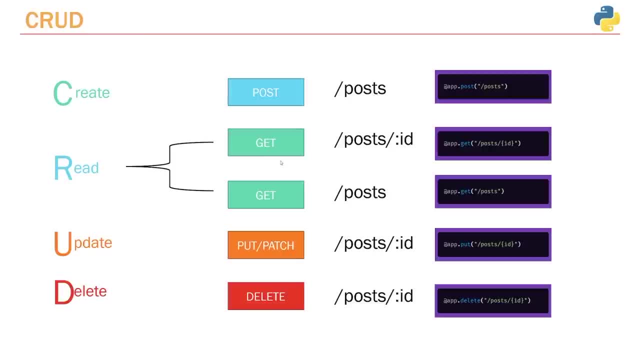 And that's if you want to get one individual post. So if we want to get detailed information about one specific post, we're going to send a get request to slash posts slash, and then we've got this ID right. So we're going to send a get request to slash posts slash, and then we've got. 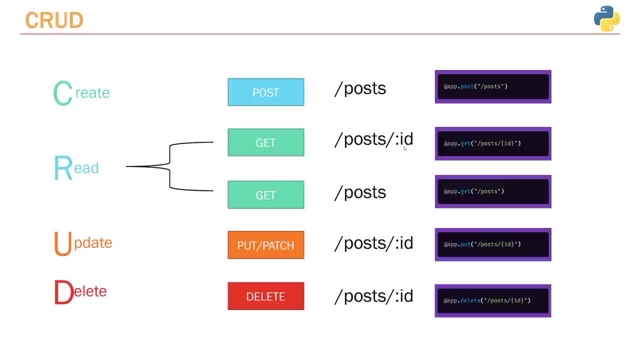 this ID right. So if we want to get detailed information about one specific post, we're going to here. So anytime you create something, what's going to happen is, anytime you add something to a database, the database is going to give it- that specific item- a unique identifier so that we can 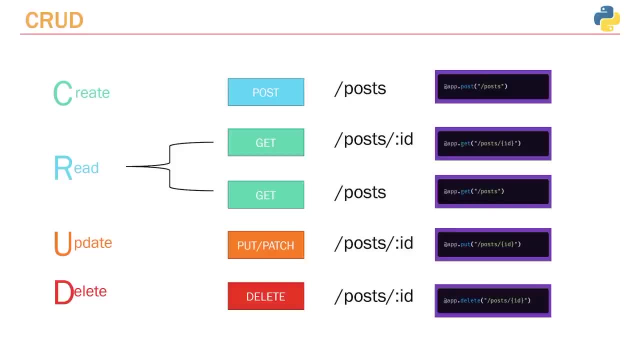 uniquely identify that specific entry, And so if I want to get detailed information about a specific post, I would just send a request to slash posts and then pass the ID of that specific post I'm interested in. So that's what this ID represents And within fast API, if you want to see what that, 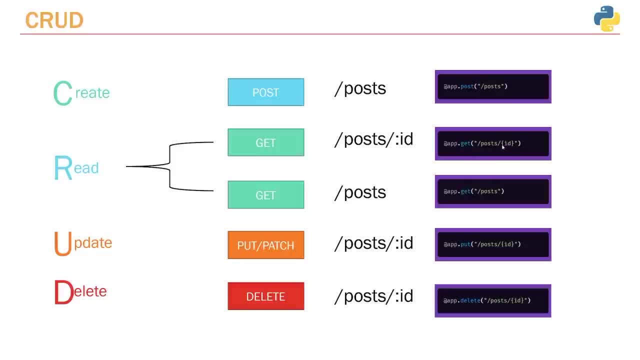 actually looks like you would just do app dot get slash posts, And then you would just send a request to slash posts, And then you would just do app dot get slash posts, And then you do curly braces and then ID, and that'll allow you to. 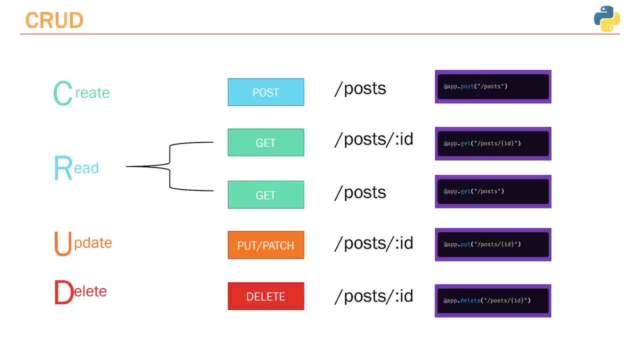 extract the ID from the specific URL of the request And then we can, you know, take that URL, sorry, take that ID, and then, you know, send it out to our database so that we can retrieve the information. So there's always going to be two specific path operations for read functionality. 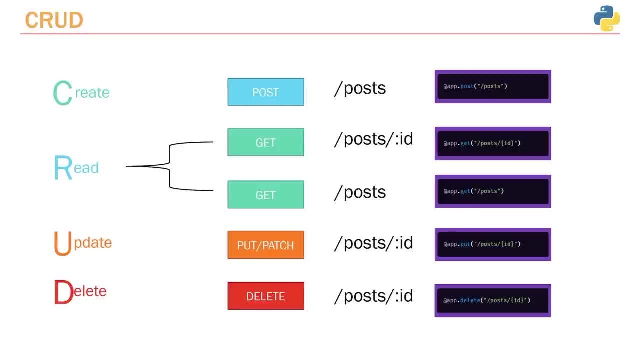 Then we have update, So this would involve updating a pre existing post. So maybe we, you know, posted out something and then we realized we said something offensive and we want to update it before anyone takes a screenshot of it. Now, when it comes to updating, 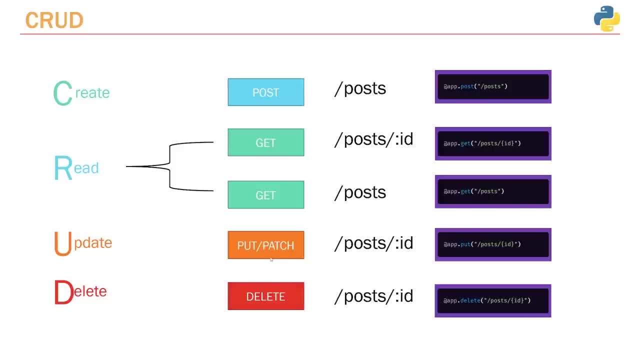 right. there's two different HTTP methods that we can use. we can use put or patch, And it's really a matter of user preference. The only difference is that I want to- I don't want to spend too much time on it- is that when we use put that you, the idea is that you pass all of the information for. 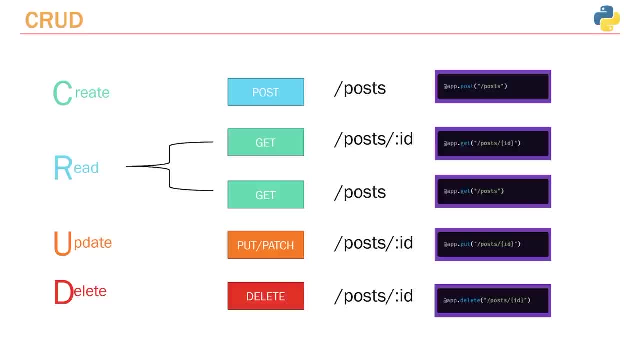 updating it. So all of the fields have to be sent to the, to the API server, whereas a patch, we can just send the specific field that we want to change. So put, change the entire thing. you have to pass every, every field, even if it's going to be the same. 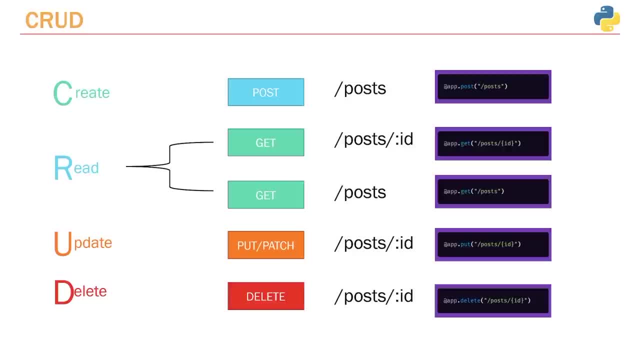 and most fields don't change, Whereas a patch we would just change that one specific field. So, as an example, as a, you know, if we're working with users, actually if we're working with posts and let's say I wanted to change the title, all right, I want to update the title of a post. 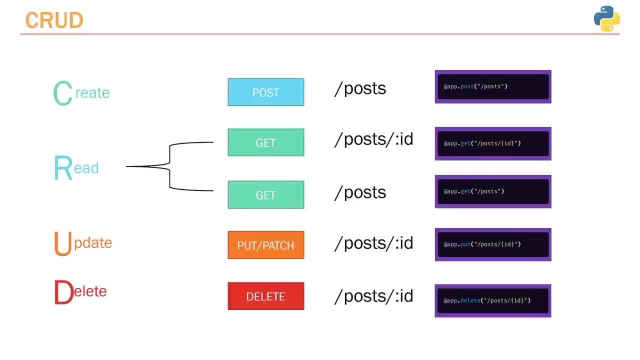 If I used a put request, I'd have to give the new title and I would have to give the pre existing content right Because the put. the idea behind put is that you have to provide all of the same information so that we can, on the back end, just take all the information and then we can update the 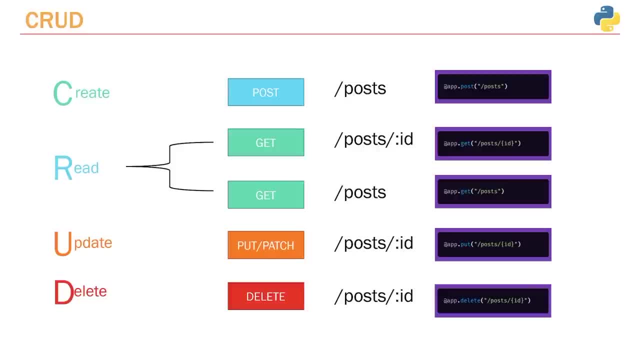 information and then update the entity, Whereas a patch operation, I can just send the title and then my back end should know how to just update that. one field We're going to stick with put I believe in our application, but really at the end of the day it doesn't really matter. 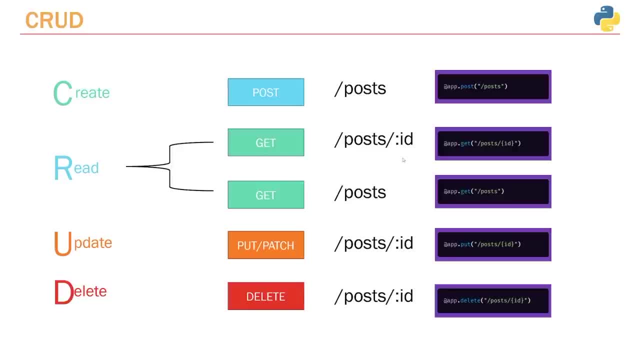 It's just a matter of use of preference. But with update, just like when it comes to retrieving one specific post, we have to pass in the ID so that we know which specific post we want to update. And for the decorator and fast API, the only thing that we change is it's going to be app dot put. 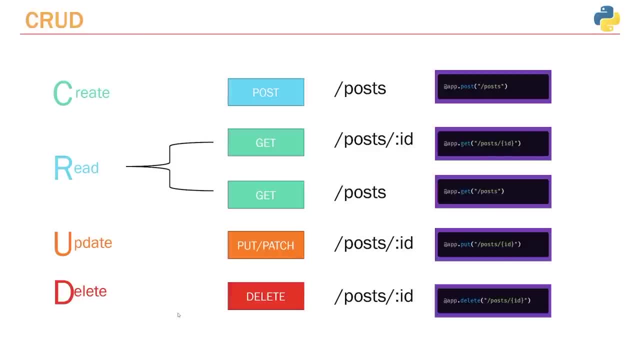 And then we can pass in the ID, like we did before, And then, finally, we have delete. So if you want to delete a post once again, you're going to send a delete request so that the HTTP verb is going to be delete, And then we have to pass in the specific ID of the post as well, And then this is what the 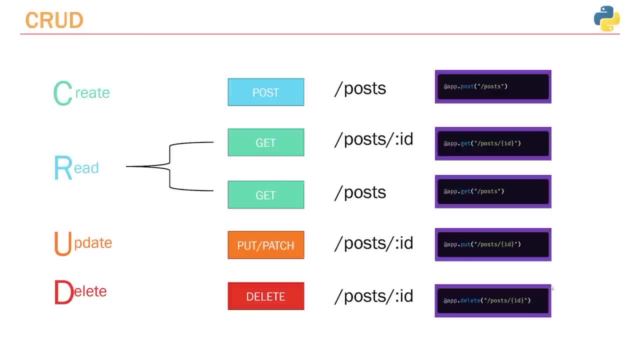 fast API decorator is going to look like. So it's actually not that hard. It's fairly simple, And you'll see that once you create one CRUD API, creating another one is almost a matter of copying and pasting, really, And so in the next video, we're going to make a few changes to our API and we're 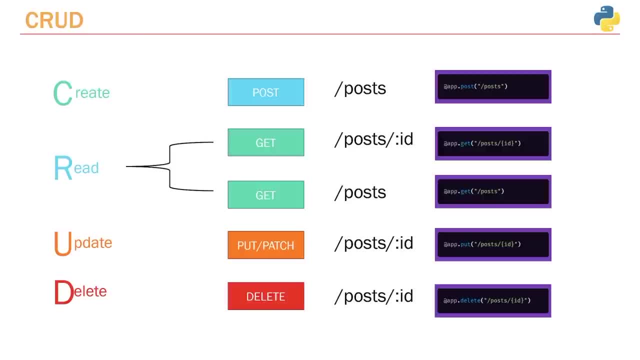 going to make a few changes to our API so that we can make sure that we follow this naming convention, because right now, I believe, when it comes to creating a post, instead of just using slash post, we called it slash create posts, which, once again, is not following best practice. So we'll update. 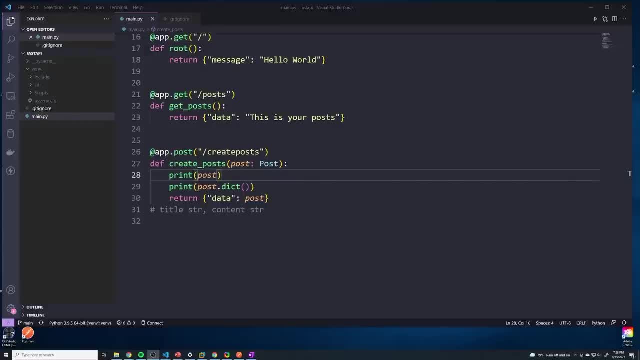 that in the next video. Alright, guys. so in the last lesson we learned about best practice and naming conventions for an API. So what I want to do is quickly go into all the code that we have and make changes so that we follow best practices. And so if you take a look at our get requests, 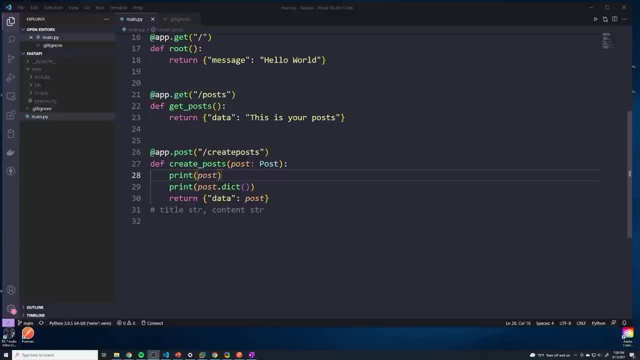 you can see we say: send a get request to slash posts- Perfect, We don't need to change anything to that. However, the issue is: is our create post functionality So the path for creating posts? we can see that we send it to a URL of slash create. 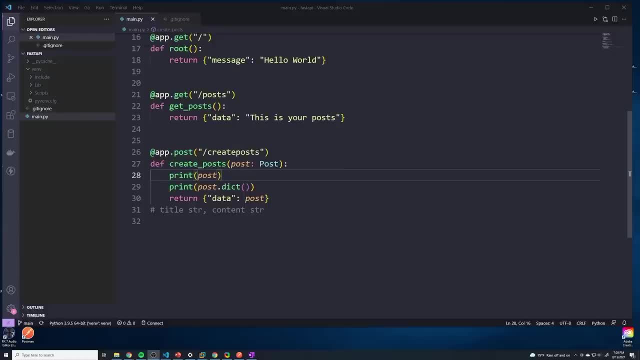 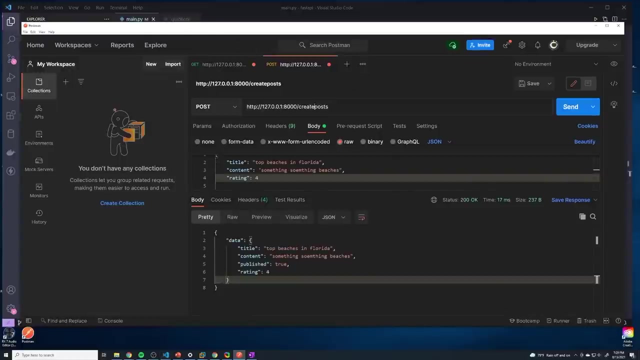 posts. that is not going and following best practice. So what we do just change this to be slash posts And that's all we have to do, And so we'll save this And we'll just double check inside our postman just to make sure we update that as well. So this is going to be to slash posts, And 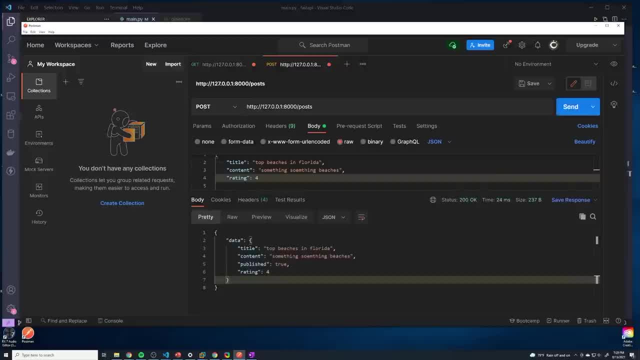 then we'll just test this out to make sure we didn't break anything, And it looks like it's still working just fine, Alright, guys. so if we take a look at our code, you can see that for our create post path function. 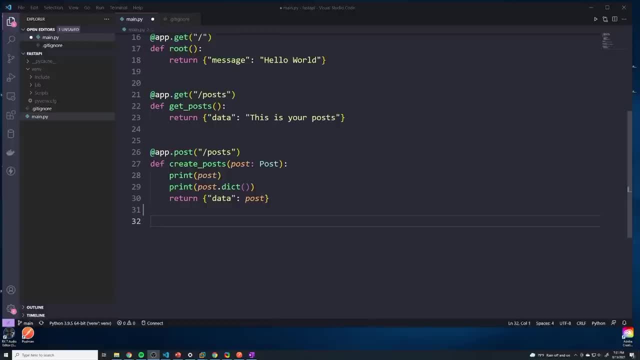 we're not actually doing anything with the data. we're not actually saving the post anywhere right now. we just print it out and then send it back to the user. So that's not exactly how a real application would work, And so what I want to do is I want to start saving these. 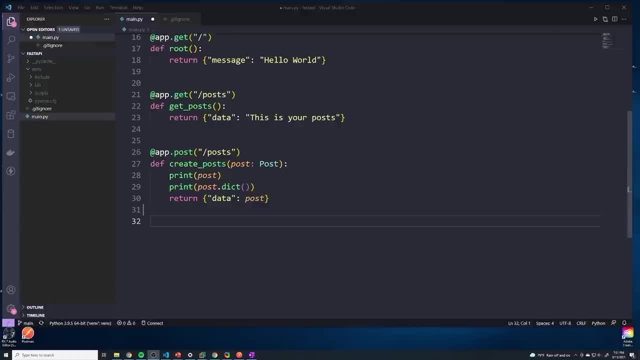 posts. I want to start turning this into a real, fully functioning application Now. ideally, we're going to save this within a database, because that's how any application works. you want to take, you want to save it in database so that you can persist that data. However, we're not quite ready. 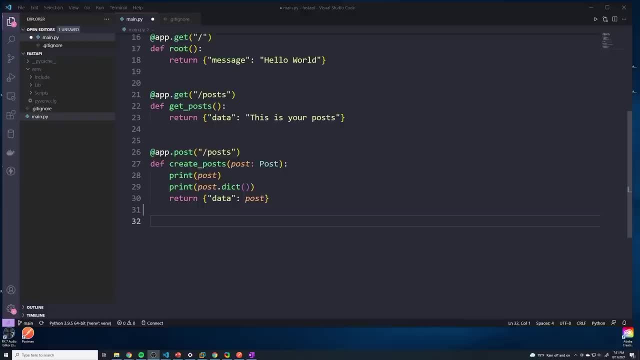 to handle working with the database. it's a little complex. we're going to get to it in this course. However, I want to keep things simple. So we're going to do is: we're going to save the posts in memory. And how do we do that? Easy, I'm just going to create a variable, just globally, that's. 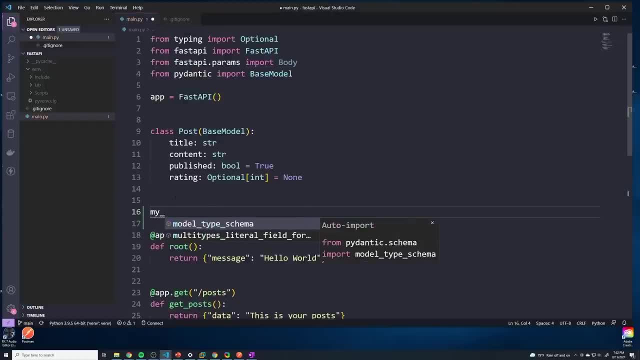 going to store all of our posts, So I'm going to say my underscore posts, And this is just going to be an array, And so this array is going to contain an a whole bunch of posts, objects, right, And what each post is going to be is it's going to be essentially a dictionary. 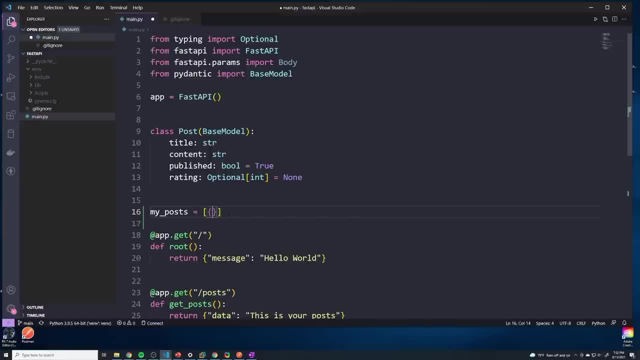 And the dictionary is going to look kind of like this: So we're going to have a couple properties, So we already know that our post is going to have a title And then that'll have you know whatever. you know title of post one or whatever. 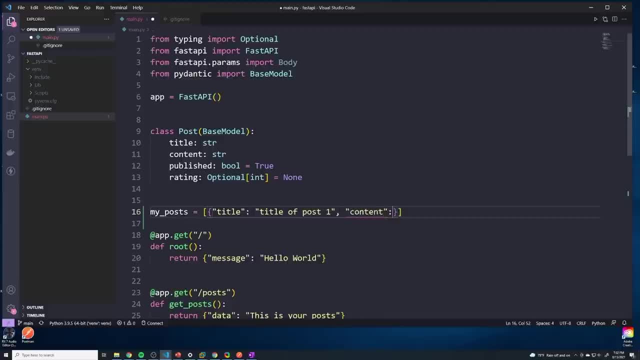 And then we're going to have the content of course, And I'll just say content of post one. This is just an example post. And then what we'll also do is, like I mentioned before, anytime you save an applicant, save a piece of information within a database. 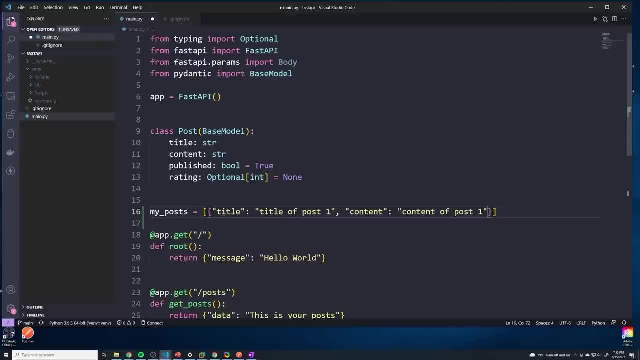 the database is going to create a unique identifier, an ID. Now, since we're not working with databases, there's no ID. However, it's going to create issues because you know, if you remember, when it comes to working with CRUD-based APIs. 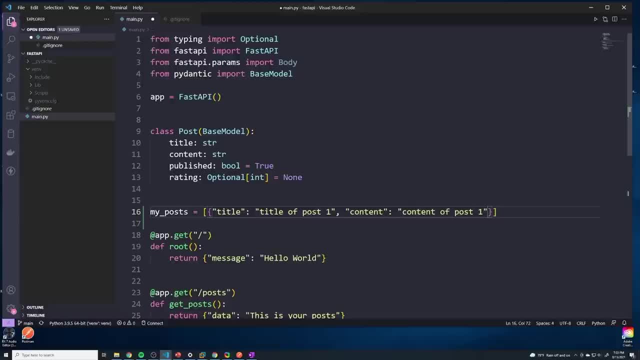 we need to be able to fetch data and update data based off of the ID of a specific post. So we do need to still have an ID so that we can uniquely reference any single item within this array. So we're going to have Another field called ID. 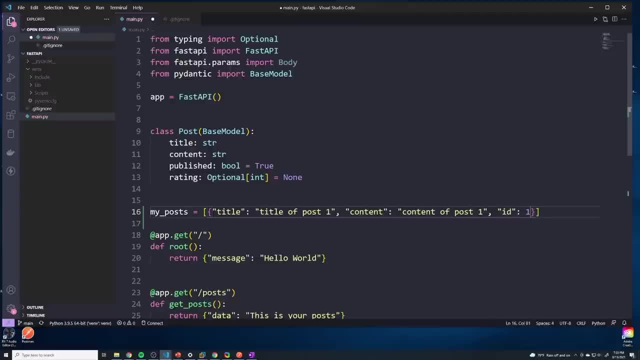 And then this is just going to have: you know, be some random integer, You know, one, two, three, four, five, It doesn't matter, It's just got to be unique. That's all that matters. So this is what our post is going to look like. 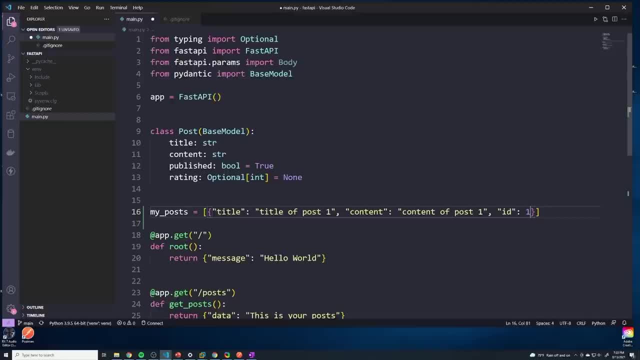 And we're going to just store it in this array. So we're going to have multiple posts And I'm going to keep this one hard-coded in here, because every time we change our code and hit save and refresh, guess what? It's going to clear this out because, remember, this is just stored in memory. 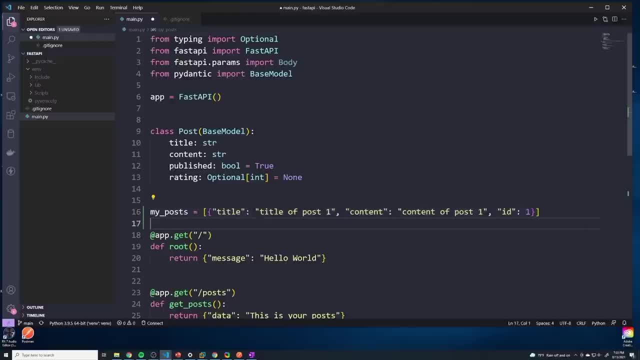 So every time our application restarts, we're going to lose that data. So just to keep things simple, I'm going to hard-code another entry. So for this post we'll say the title is Favorite Foods And the content will be: 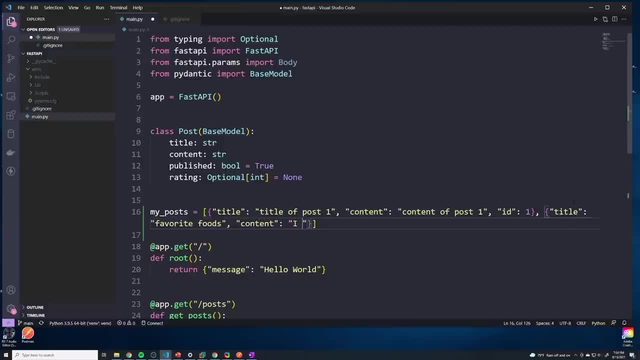 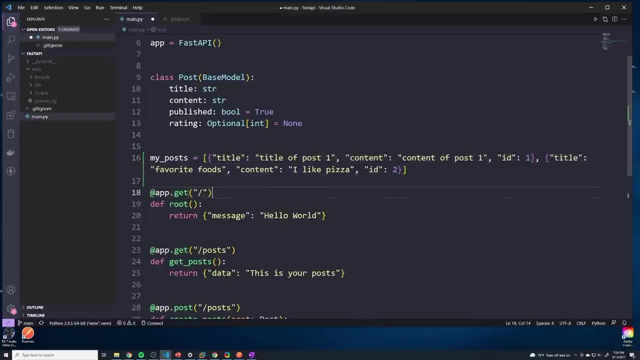 I Like Pizza And we'll just give this an ID of two. All right, And so now that we actually have some place to store our post, we can actually test out our get post functionality to see if it works. So I'm going to save this. we're going to go back. 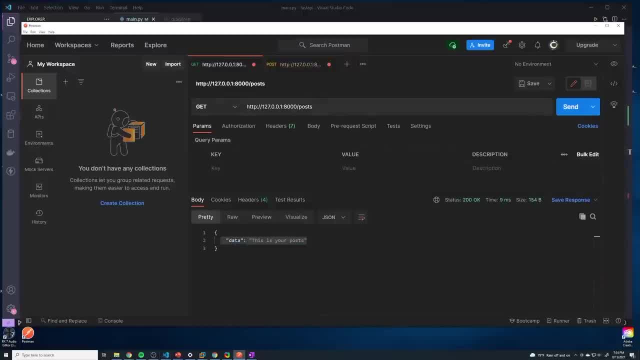 to postman. So find the one with the get operation where we're retrieving the posts, And then we'll hit send. Let's see, Well, when we hit send, nothing happens, of course, because we actually have to update the code to send that data. So let's go back to our code And let's go to our 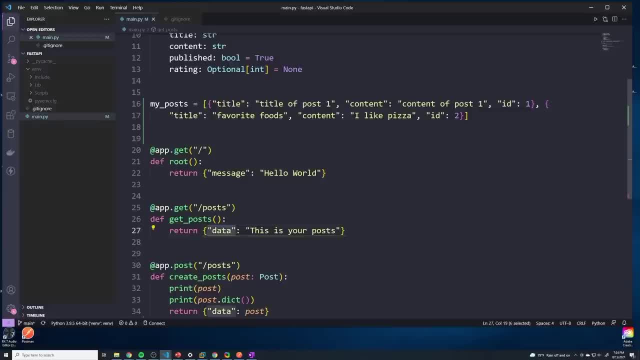 get posts, So right now we're just sending back this information, So let's update this so that we return my posts, And this should be fairly straightforward. what we can do is we can just keep this property called data, And then we can just remove this and just pass along my underscore. 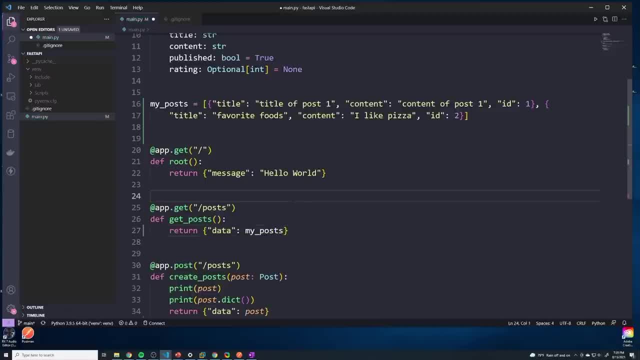 posts, And so what's going to happen is fast. API is great, because if I pass in an array like this, it'll automatically serialize it, So it's going to convert it into JSON. JSON has something that's also very similar to an array, And it's going to change that into a JSON format so that we can send. 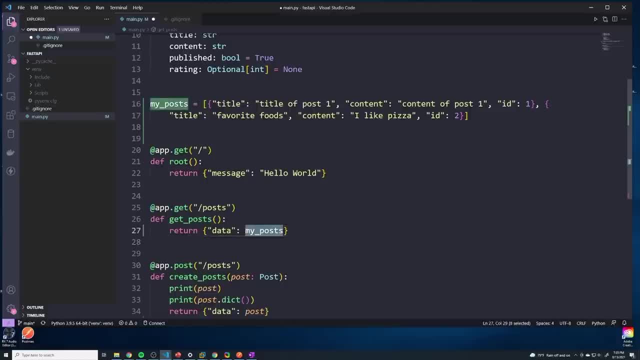 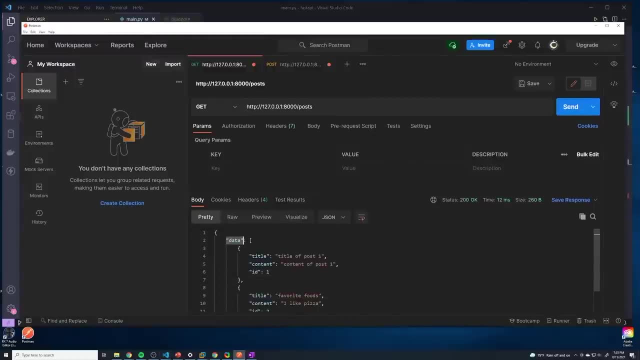 it over our API. So that's all we have to do. we just have to pass in the array And it's going to send that. Now, if we try this, look at that. So we get the data property And within here: 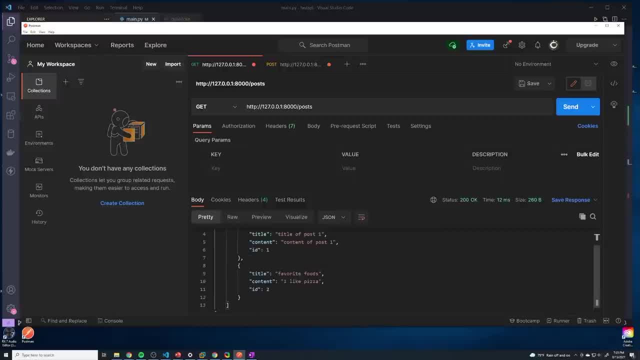 we have an array. So this is JSON also has a concept of arrays- And then within here you can see we've got our post one and our posts too. So that's really as simple as how to work with our API, how to actually retrieve posts. In the next video we're going to update the 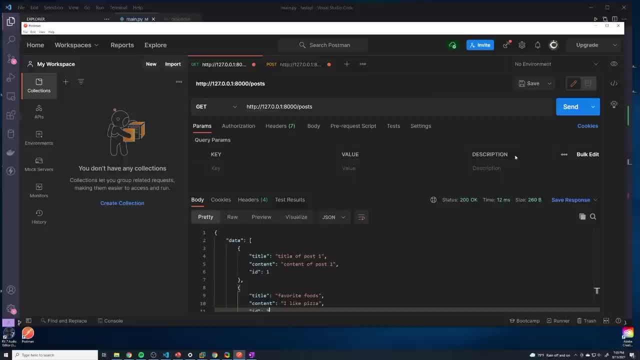 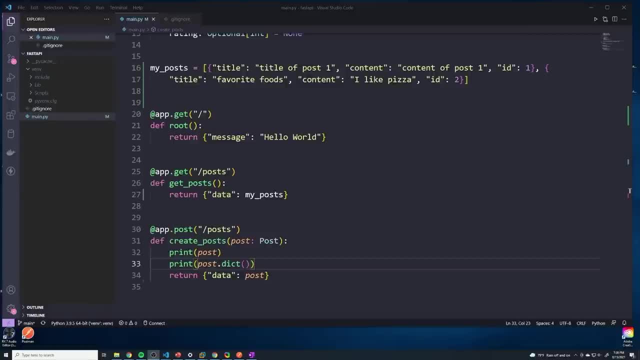 create post path operation so that we can figure out how to add a new post into our my posts array. All right guys. so let's update our create post path operation function so that we can retrieve the title and the content from our front end and then create a brand new post and 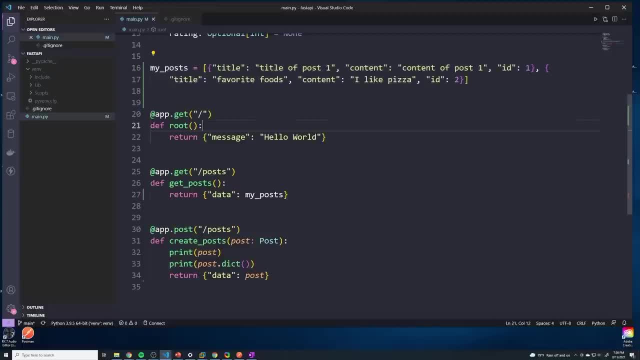 store it within our my posts array. So how do we do that? Well, we already know that we can retrieve our post by referencing this post variable, because this will take our schema which, remember, we defined with pydantic, it's going to do all the validation and it's going to store it. 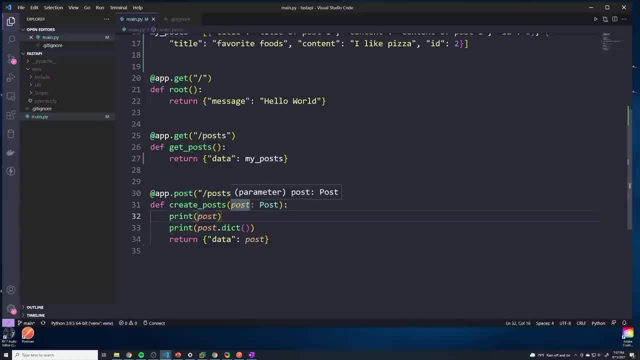 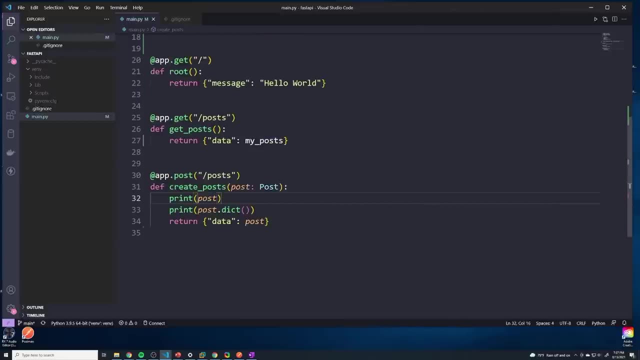 within post, And so this is still going to be a pydantic model. However, our our array is going to be an array of dictionaries, So we have to convert that to dictionaries, And we already know that we can convert any pydantic model to a dictionary by doing dot, dict And then that'll. 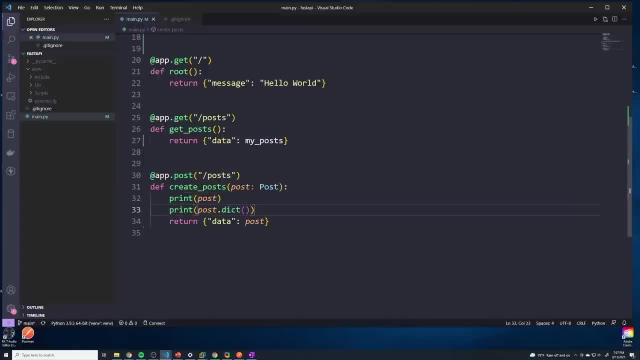 turn it into a standard Python dictionary, And at that point it's pretty simple. This is just standard Python. At this point we can just do a my underscore posts dot append, And then we can append post dot dict, Just like we did before. we don't. we can remove these print statements, they're just. 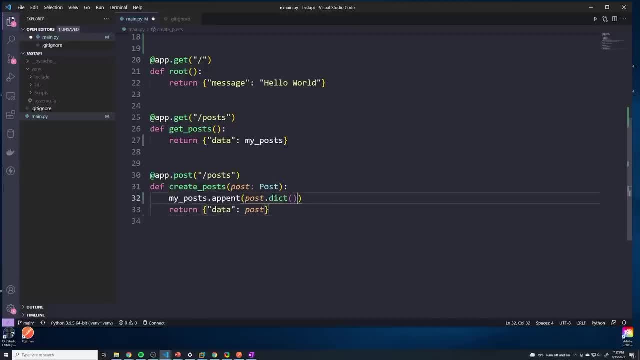 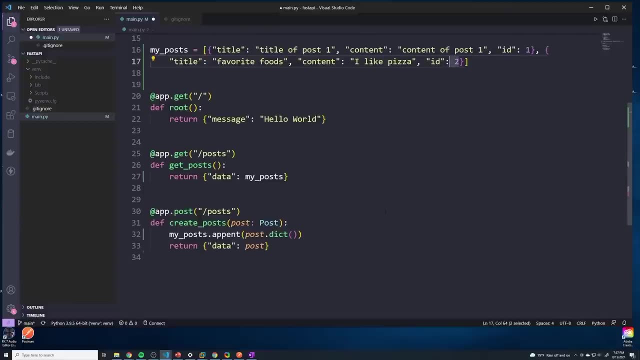 cluttering things up. However, there's one little issue. Like I said, we need to have an ID for every entry, And normally the database handles that. But since we're not actually working with a real database, we're going to have to do this in software. So what I'm going to do, 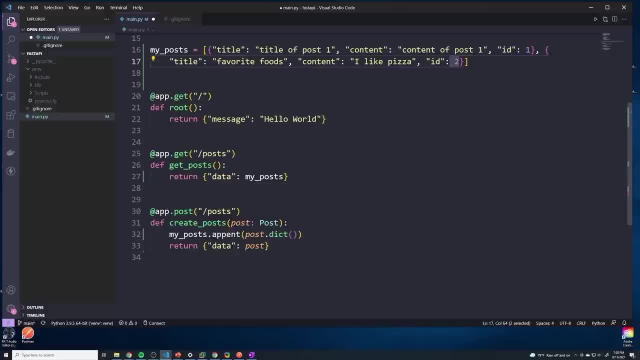 is we're just going to assign it a random integer. not really that reliable, But if we pick a random number between one and, you know, 10 million, the odds of us hitting the same number twice is almost next to none. So what we're going to do is we're going to use the random package. 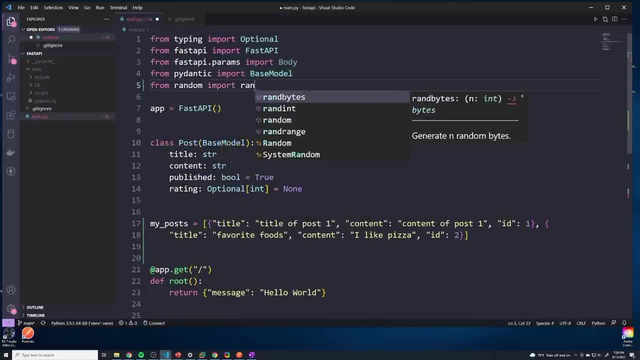 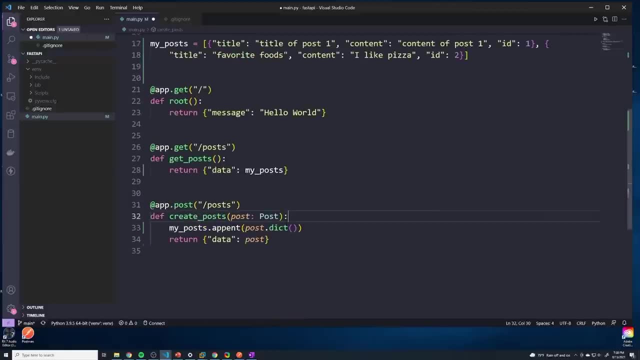 So we'll say, from random import ran range, and this is what we're going to use to create a random number or a random integer. And so, instead of doing this, I'm actually going to remove this for a second, And I spelled append wrong as well. What we're going to do is I'm going to say post underscore. 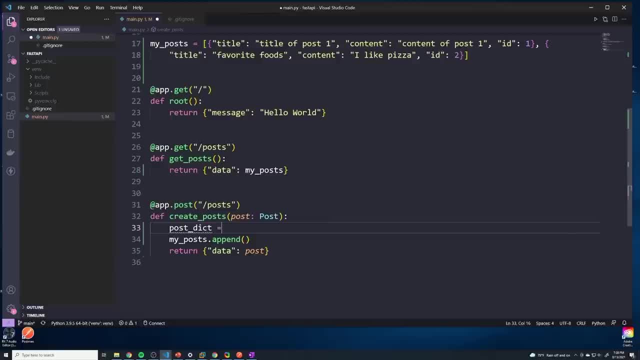 which is going to be the post pydentic model converted to a dictionary. I'm going to set that equal to post dot dict. Okay, so this is going to be the dictionary, And so now that we have a regular Python dictionary, what we can say is post underscore- dict. And then I'm going to reference: 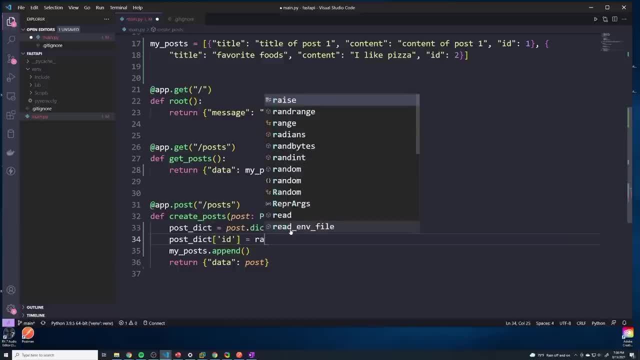 the ID field that I'm creating And I'm going to assign that to be a random number. So we're going to give it a range of zero to and then just pick some really, really, really, really large number. So this is going to ensure that pretty much any entry won't. 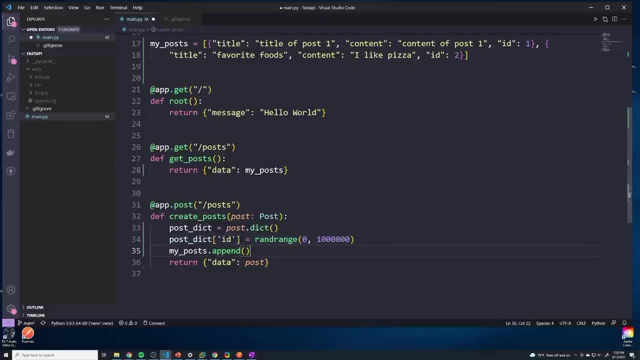 for development purposes is going to be unique, We'll append that to the array. And then here's the thing when it comes to how a usual API works is that when a front end sends the data to create a new post, after we create the post stored in our database, we should send back the newly created. 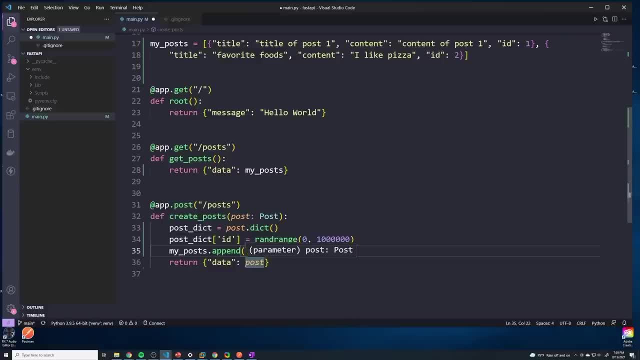 post including the brand new ID, So let's send that back. So in this case, I'm going to send back post underscore dick, because that's going to be the brand new post that we add to the specific add to our posts array. So let's try this out. Let's go to our post request that we have. 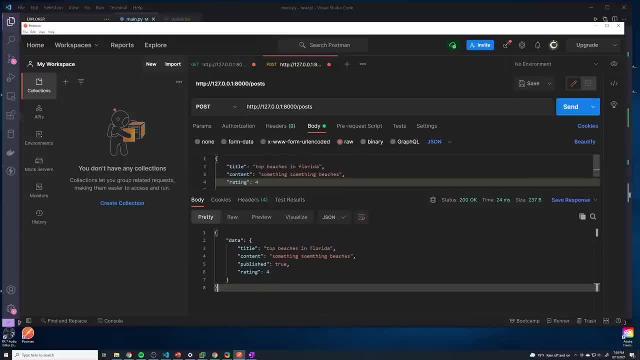 And let's see all of our data. So we've got a couple of things: title, content, rating- I don't really care about the rating, But I'll just leave it in there- for now it shouldn't matter- And then we'll just hit send And let's see what happens. And it looks like we got. 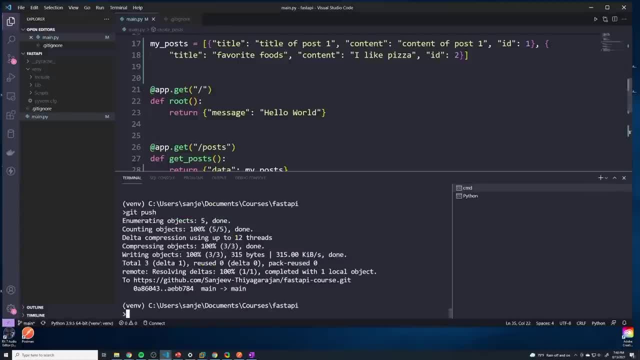 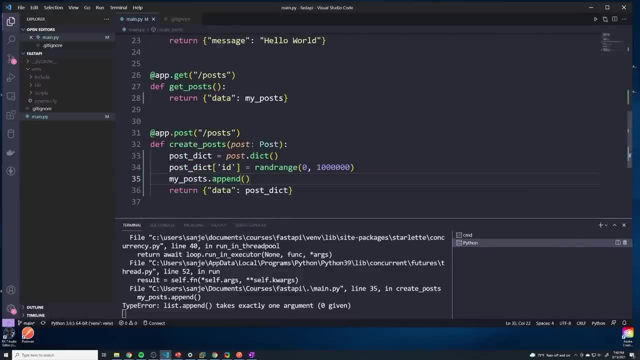 it in there for now, So let's go ahead and hit send And let's see what happens. And it looks like we got an error, So let's see what happened. It looks like there's an and I already see what happened. I forgot to actually include. 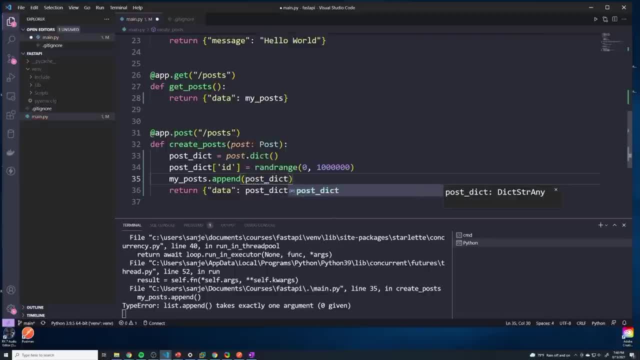 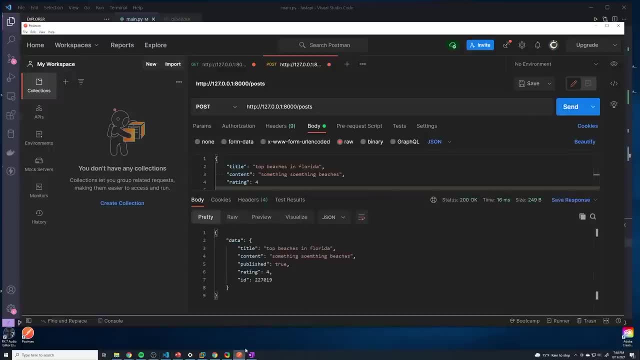 post underscore: dict. We actually have to pass in what we want to append to the array. Let's save that. Try this again. hopefully no errors. Look at that guys. So it looks like we got back the newly created entry And if we can see that it has an ID of whatever that number is, And if we 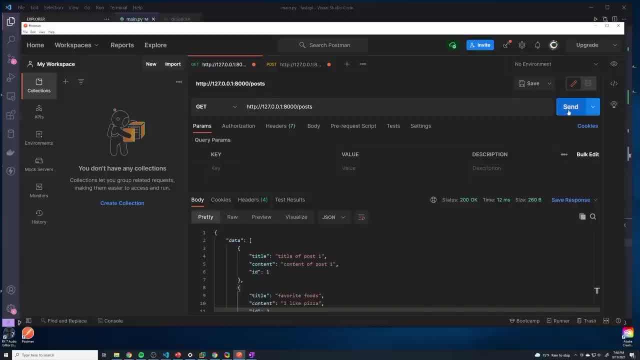 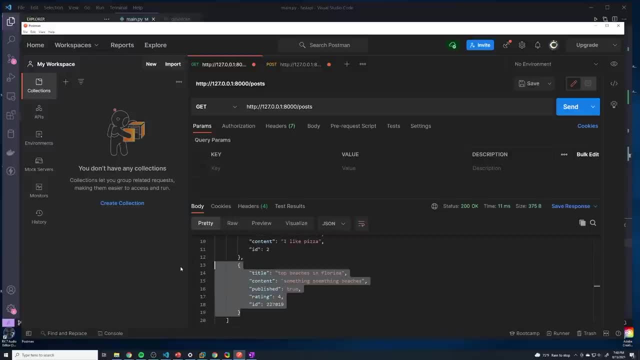 do a get request now to retrieve all of our posts? we should see that newly created entry. So let's take a look. We've got post one, post two And then we've got that brand new post. Look at that, guys. 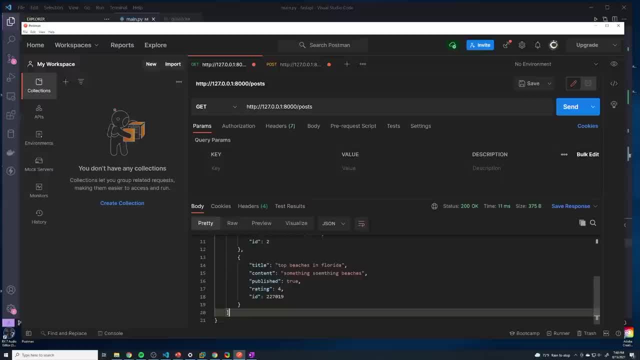 So we are a little bit less than halfway done with creating our crud based application. Now, before moving any further and writing any more code, what I want to do is I want to actually save these requests, because right now they're just kind of stored in memory If we close out. postman, it'll still remember it. But what we can do is we can create a code that we want to save. So let's go ahead and hit save And if we close out, postman it'll still remember it. But what we can 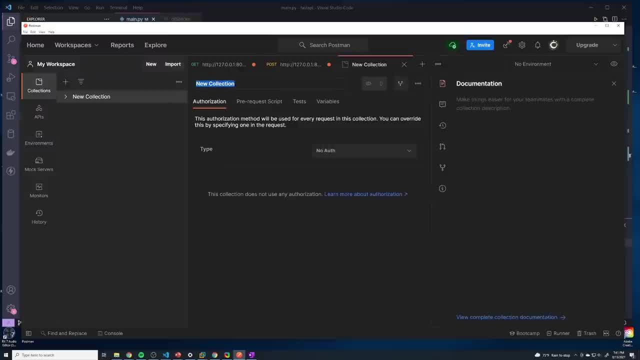 do is we can create a collection. So here I'm going to select, create collection And I'm going to give this a name. So I'm just going to name this after my project. So I can call this, you know, fast API course or, you know, since this is a social media app, we can call it whatever we. 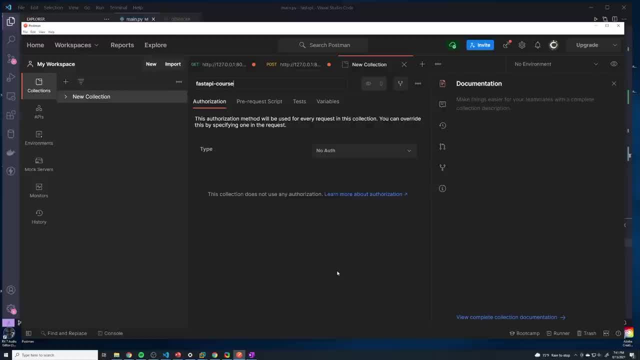 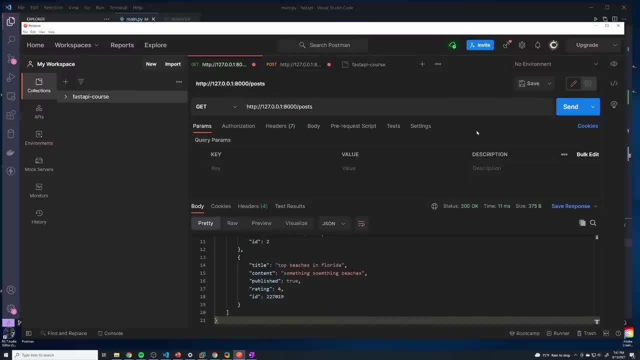 were to call it. I'm just gonna call it fast: API course. we'll save that. And then what I want to do is I want to save these two requests so that I don't have to remember this in case they actually get deleted. So I'll hit save- save, as we'll save it, and then you can give it any name. So this is. 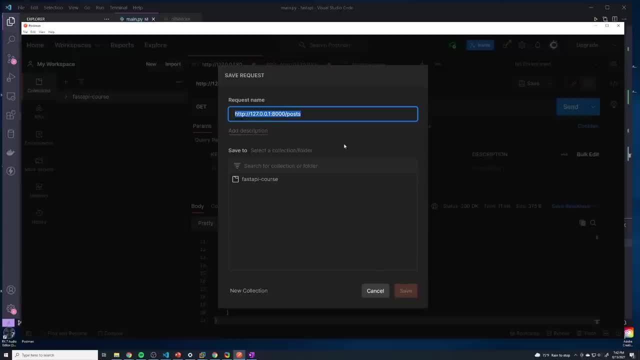 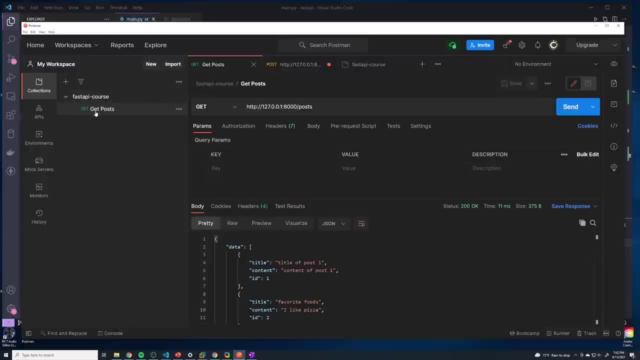 going to be. I forget, this is the get request. So I'm going to say I'm gonna call this get posts and I stored inside this collection And so now within this collection, you can see this request is stored in there. I'm gonna do the same thing for the post request. So this is for creating. 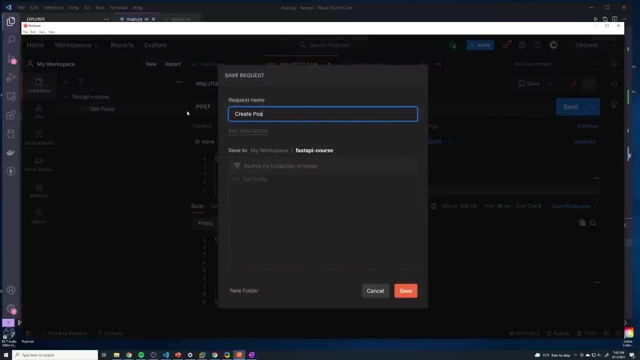 posts. we'll do save, as again I'm going to say create post And then it's already remembers the most recent collection. but go ahead and select the collection if it didn't remember that, And then we'll hit save And so now they're both saved in here And we can easily bring these up anytime. 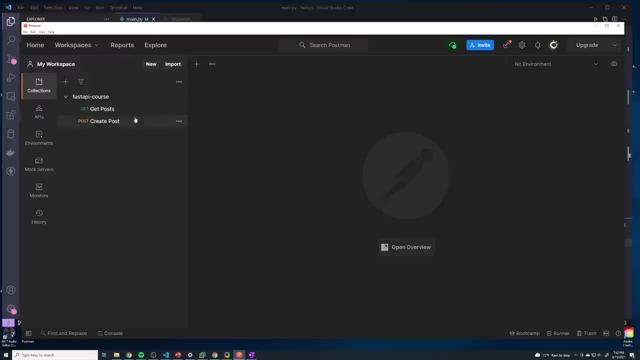 even if we close out all of our requests. So I closed everything out and bring that right back up. it's going to remember everything. And then same thing with the post request. I go to the body. it even remembers the fields. So, postman, one of my favorite tools when it comes to working. 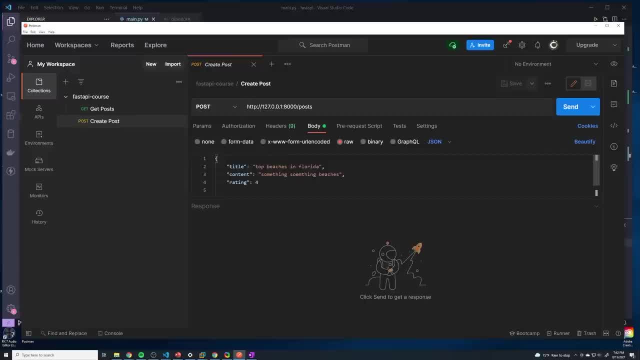 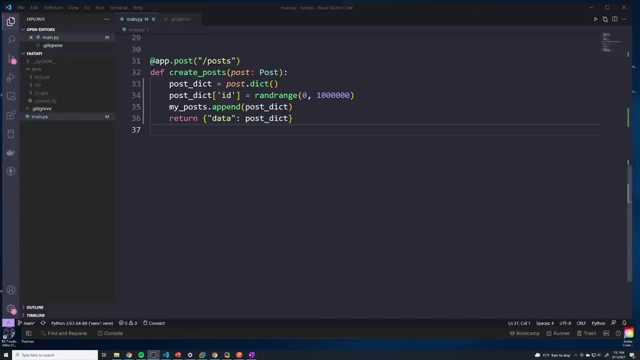 with API's And you know, as this course goes along, you're going to continue to learn more and more things about postman. Okay, guys, let's continue building out our CRUD application. The next function I want to implement is retrieving one individual post, And so. 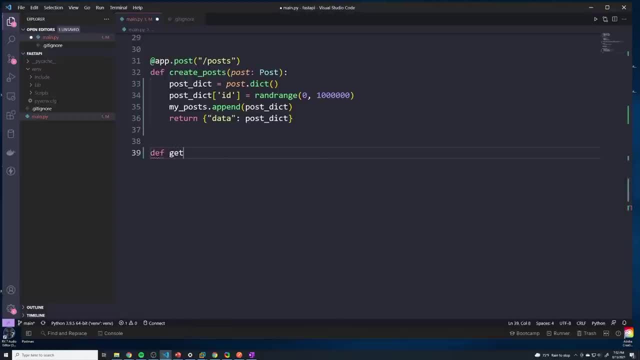 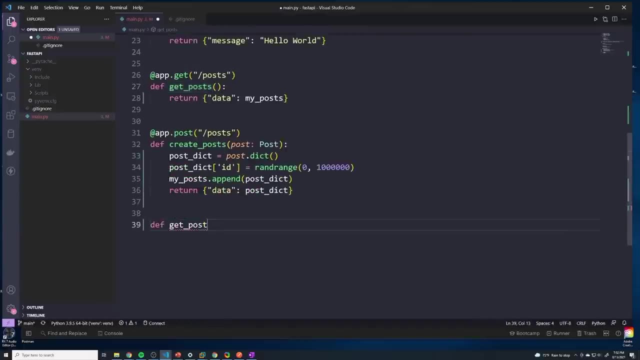 let's define a function for that. So here I'll call this get post. Keep in mind that this is singular, So I call this get post, whereas to retrieve all posts it's get posts. But, like I said, the name of these functions don't actually matter, It's just more for for you, more for. 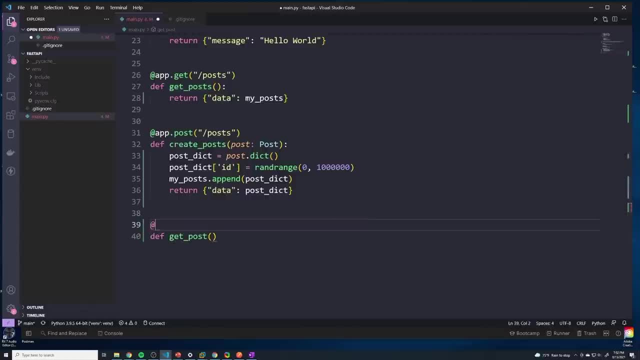 readability And the decorator is going to look like this, And so this is based off of that slide I already showed you. So it's going to be a get method, And then here the URL is going to be slash posts ID, right, because the user 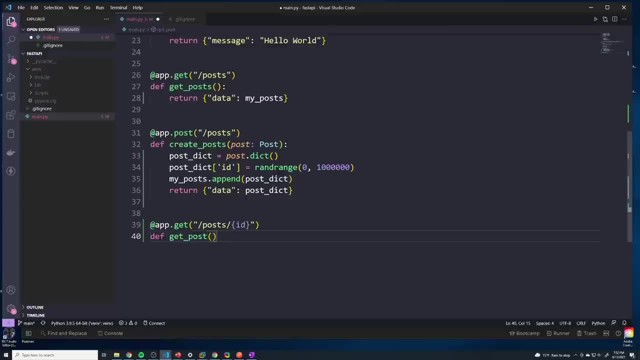 is going to provide us the ID of the specific post that they're interested in, And so that's going to get embedded in the URL. So they'll send a get request to slash, post slash and then whatever ID. So if they want to see the information for post one, they'll pass in a value of one And 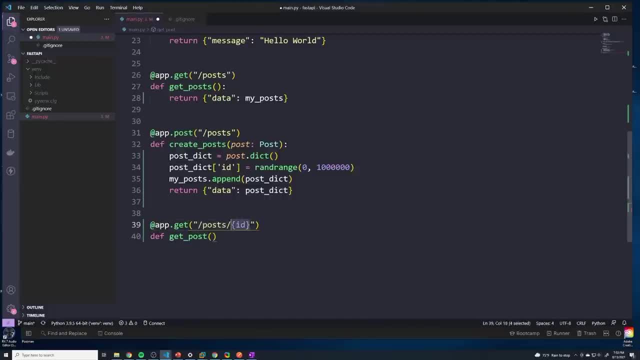 what this is actually referred to. the proper terminology for this is: this is called a path parameter, So this ID field represents a path parameter, And this parameter happens to represent the ID of a specific post, the user's ID, So this is called a path parameter And this parameter. 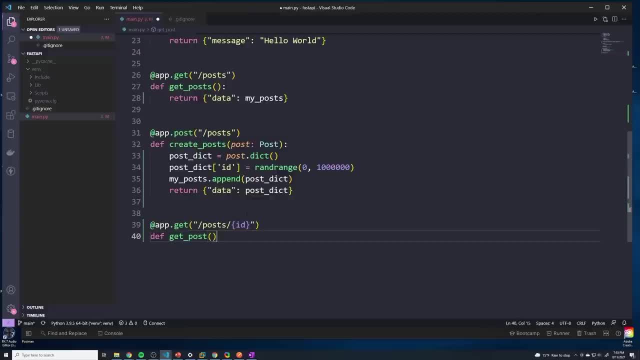 is the one that you're interested in seeing, And so what we can do is fast. API will automatically extract this ID, and then we can pass it right into our function. So now our function has access to whatever value was in that URL right there, And so, if we want to, I can do a quick. 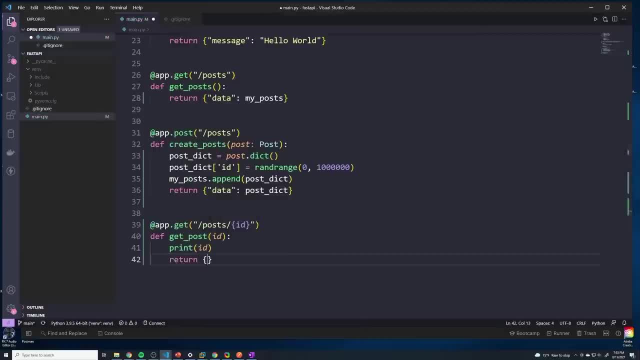 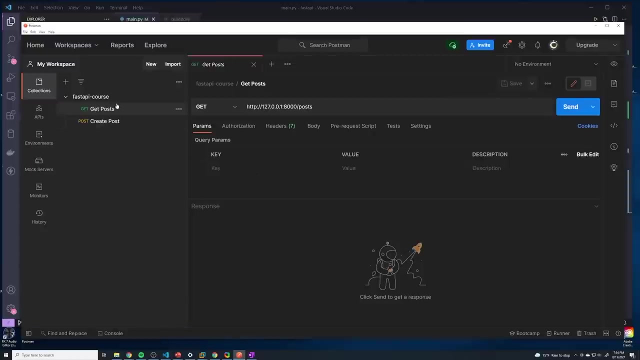 print of ID And then we'll just return some hard coded data. So I'll just say data And we'll call this a how about post? underscore detail: I'll say this is the post you're interested in. Or even better I can do is we'll change this to an F string And I'll just say here is post, And then we can just pass an ID. So let's save that. We'll go to postman And what we want to do is we want to create a new post, but let's create it in our collection. So I'm going to go in there, select add request, give it whatever name you want. I'll say get one post And then for the URL, just copy the get posts URL. 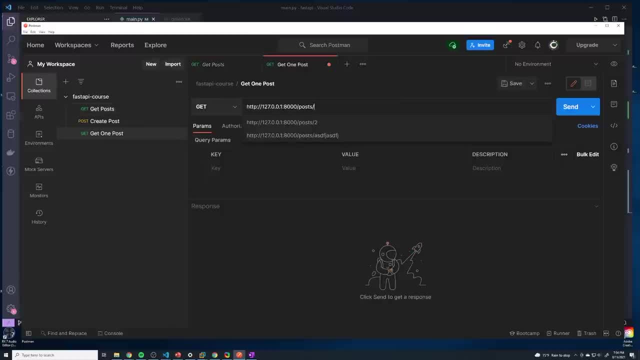 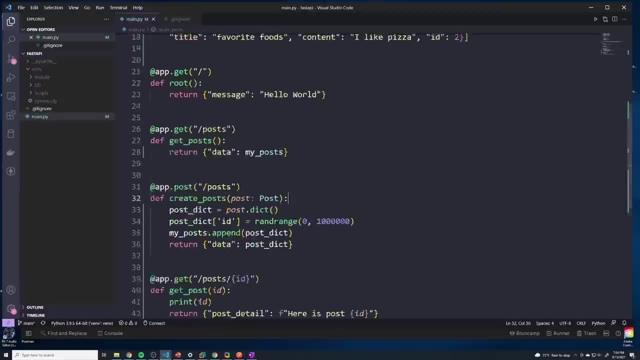 And then we want to pass in the ID that we're interested in, So we just do slash, And then, in this case, I'm going to get the post with an ID of two, And the reason why I'm doing that is because we've hard coded one of our posts to have an ID of two, So I know that's always going to be there. 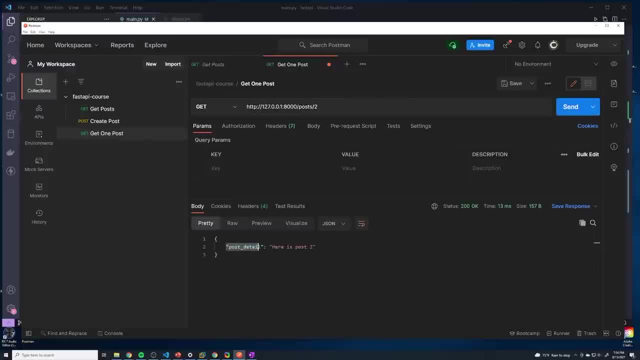 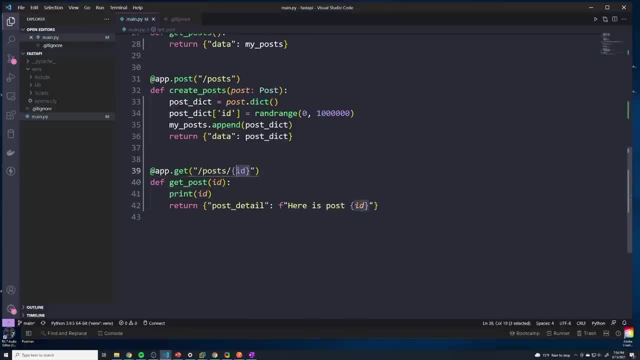 And then we can just try sending this and see what happens. So it says post detail, here is post, and then post number two. So it looks like we were successfully able to extract the ID, the path parameter that was passed into the specific URL that the user sent a request. 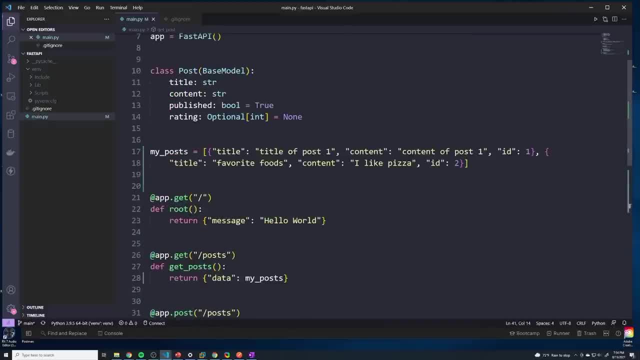 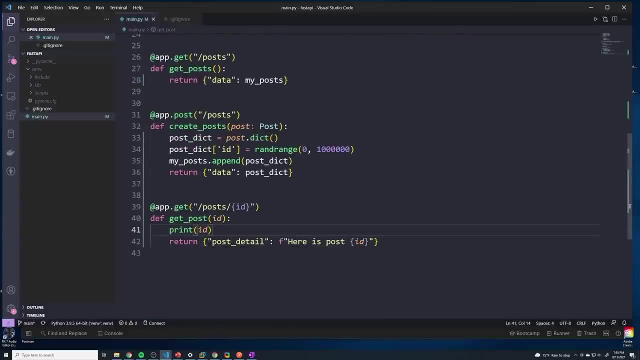 So we now have access to that. at that point, we can just find whichever entry in my posts has that specific ID. Now we have to implement the logic for actually getting that post, And so there's many different ways of doing this, And I'm telling you right now this is probably not the best way of doing this. I'm not really even a Python expert. I'm sure there's much better ways of grabbing this information. However, keep in mind, the code is going to be changed later on, once we start working with the database. So this, at this point, is just basic Python logic, And I do want to keep 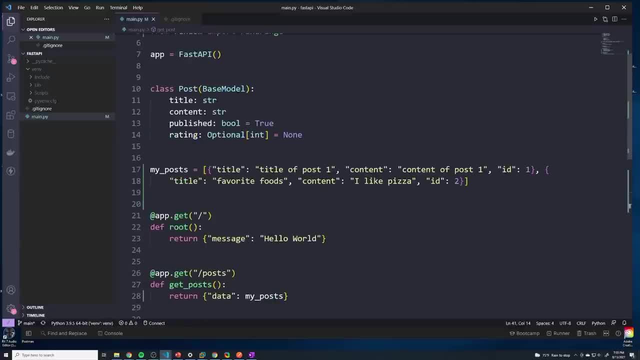 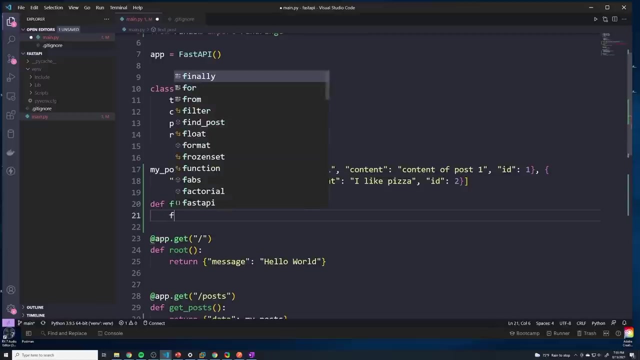 I do want you guys to keep in mind that this may not be best practice for the best way of retrieving an individual post, but I'm just going to create a simple function And it's going to be called find posts. So this is how you find a post: by an ID, So the. so we'll pass in an ID in this function to retrieve the post, And what we'll do is we'll iterate over the my posts. we'll say for P in my posts And we'll say if P, so P represents the specific post that we're iterating over. So if this, 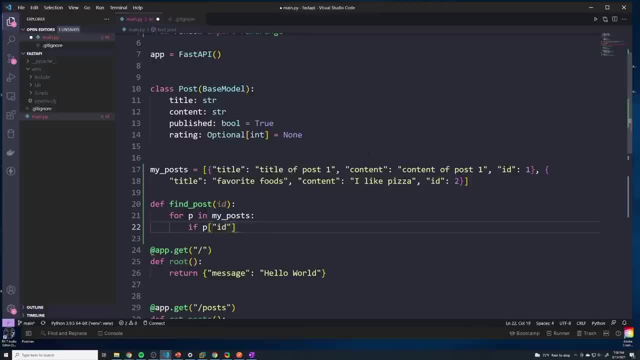 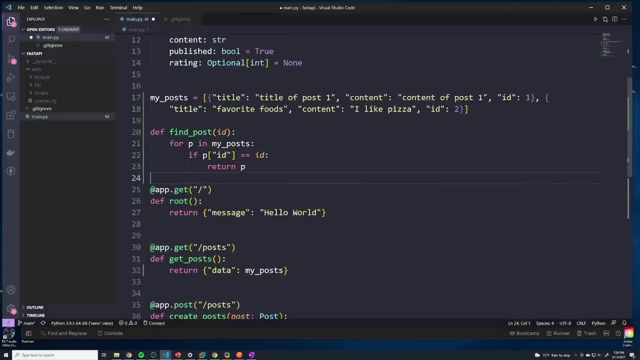 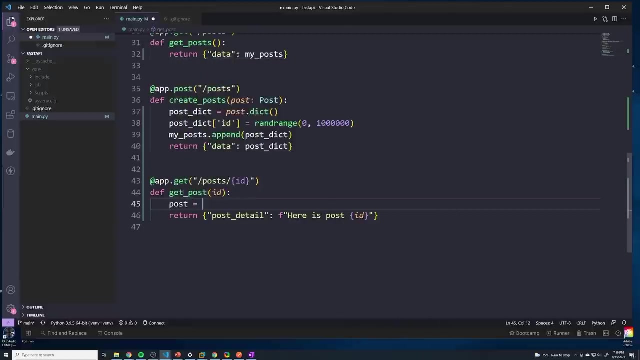 specific post has an ID which equals the ID that was passed into the function, then we'll return P or return that specific post And then at this point we can call this function. So I'm going to remove that print statement and say post equals, find underscore post ID And then for: 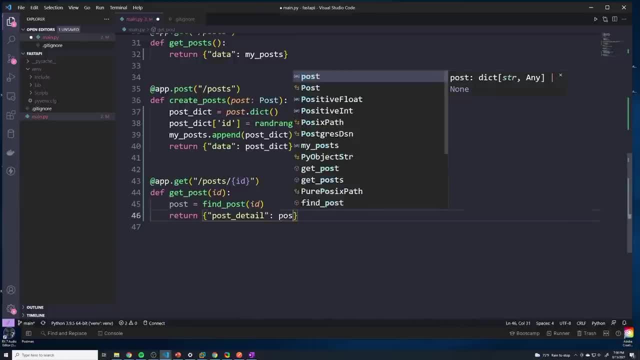 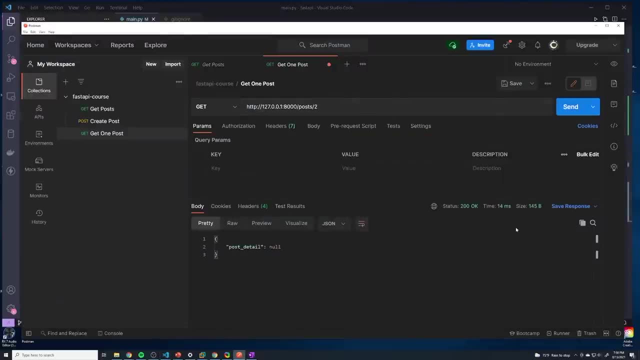 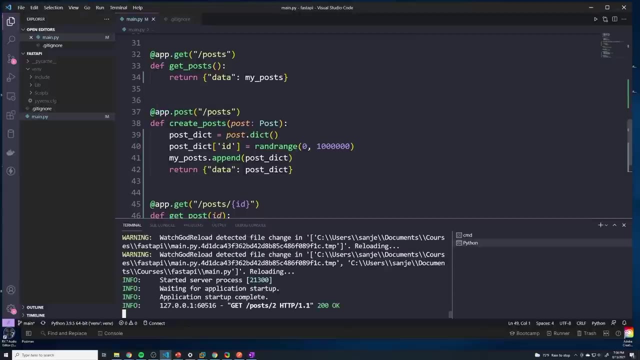 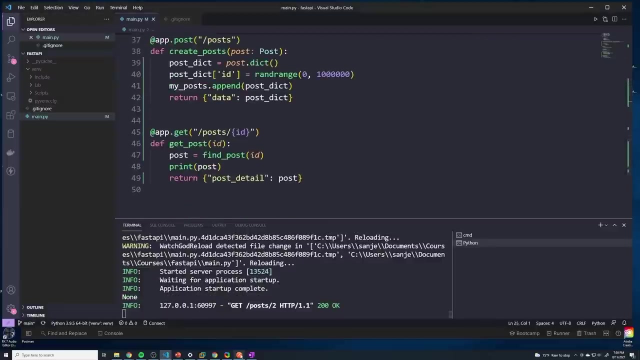 this. we can just remove this and just return post. Let's save this, let's go to back to postman And let's try this out. And it looks like I got an error. So something happened And let's actually take a look at our code. Well guys, I think I found the issue. So the reason why we keep getting none right, If I keep sending, sending, send, it says none. And what I did was I just printed out the post to see. 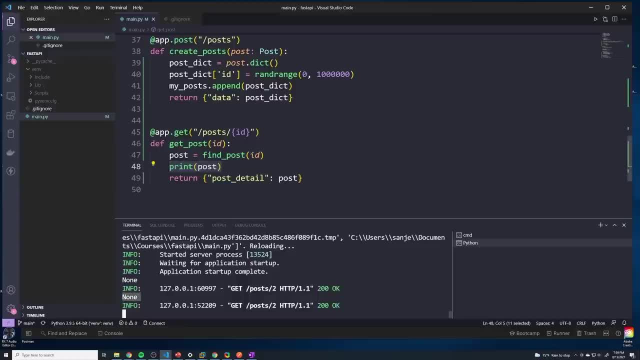 what we got, And it actually just prints out none. So if, for some reason, we're unable to find posts- and I think I know exactly why, And so what I'm going to do is I'm going to do a print of ID again, And this is going to teach us an important lesson. So I sent. 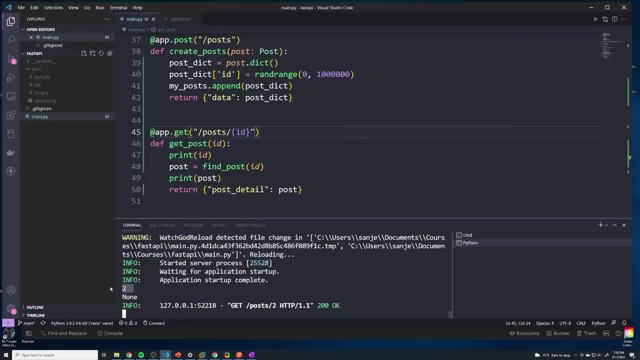 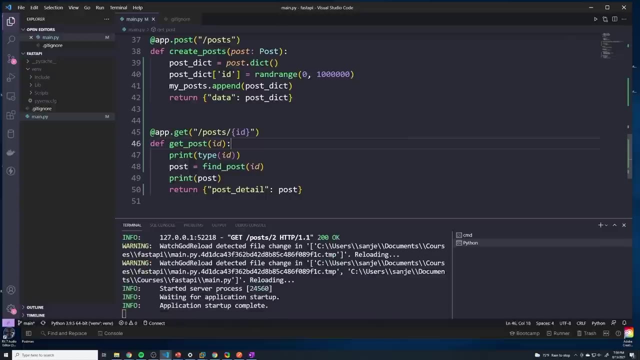 another request And it prints out to. however, what we're going to do is I'm actually going to get the type of ID, So I forget how to do that. I think it's the type, like you could just do type in Python, So I'm going to figure out what is the actual type of ID. And now, 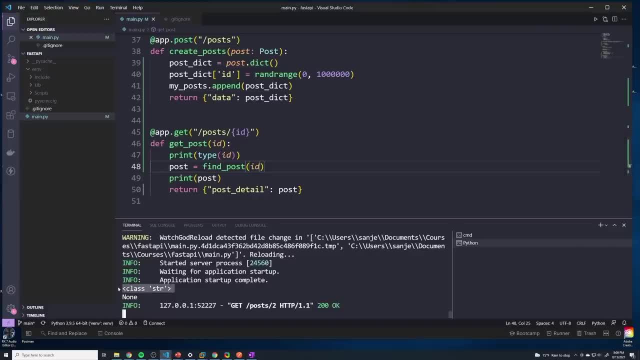 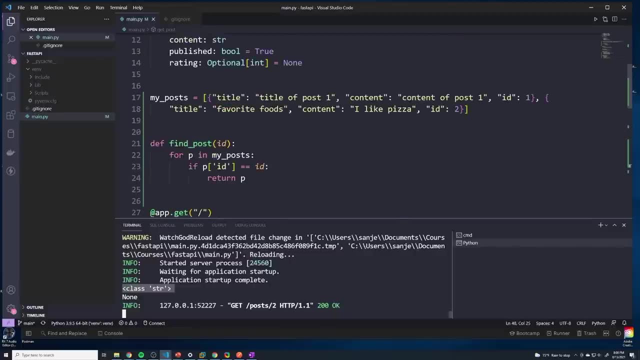 if I send this request again. right, you could see that the type is actually a string and not an integer. And so when we pass this check in where we say if P ID, so if we get the ID field and compare it to the ID that we pass in, it's never going to equal that, because 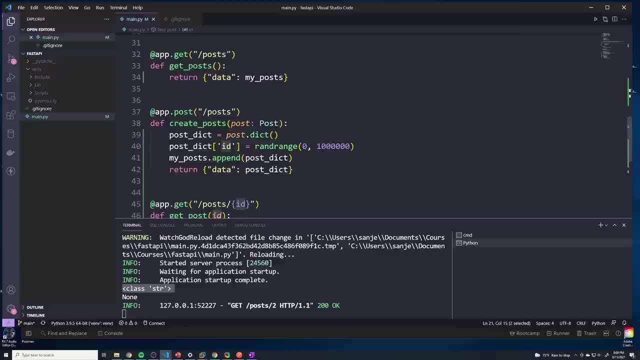 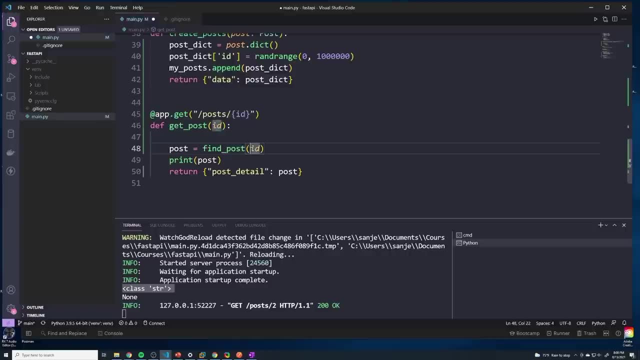 one's an integer, the other one's a string. they're never going to be equal. So the first thing that we actually have to do is, before we call this function, we have to convert it to an integer. So I can just say: int, that's going to convert. 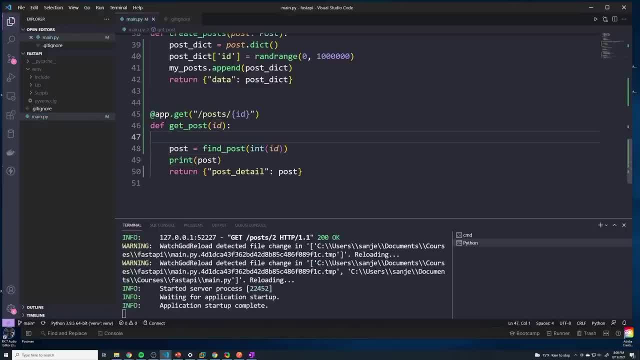 it to an int, Save that, And then, at this point, if I send this, it should now work. Look at that. So keep in mind, guys: anytime we have a path parameter, it's always going to be returned as a string, even if it represents an integer or a number. we always have to. 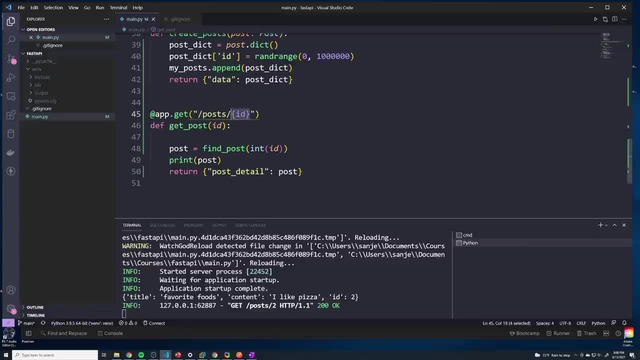 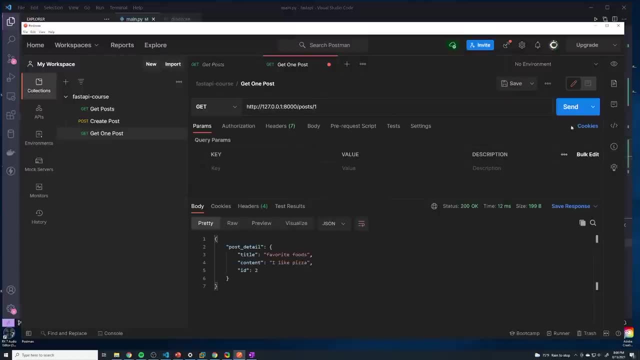 manually convert it ourselves, So don't forget to do that. Now there is one little issue with what we're doing, So everything's working, And if I actually change this to a one, we should get a different post. So everything's. 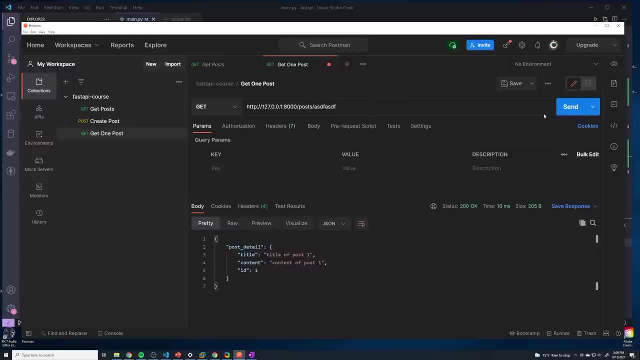 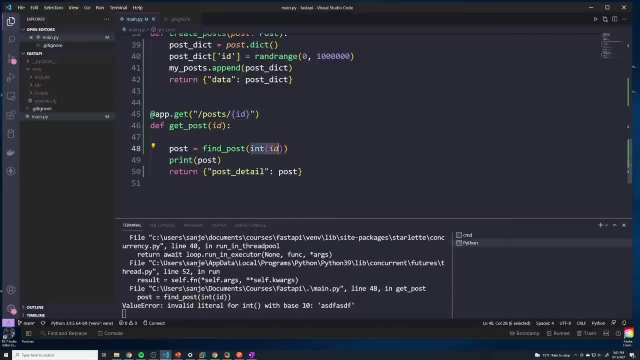 working great. However, what happens if I type this: Well, let's hit send. Well, we get an error right Because we're trying to convert this to an int And it's going to throw an error. And then, instead of sending back a nice you know, built in response. 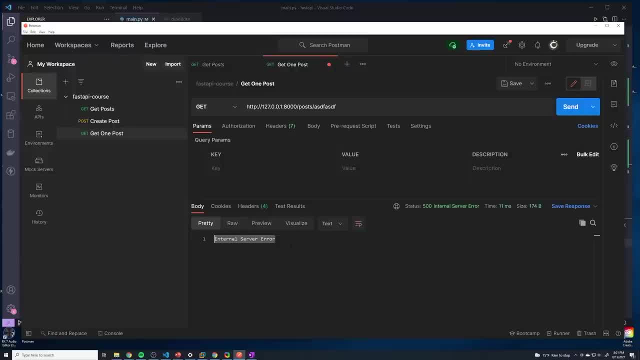 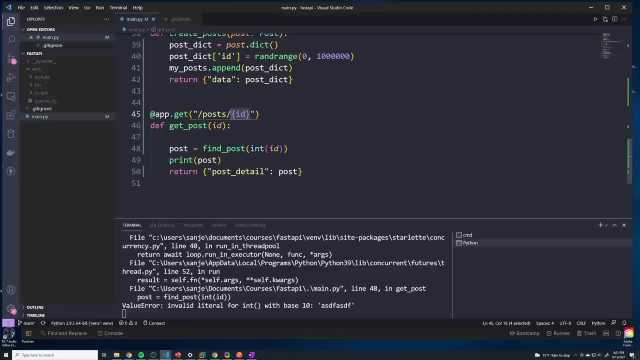 we just get an internal server error and the user has no idea what exactly is wrong. So we want to provide feedback. So how can we perform some kind of validation to ensure that whatever data that's passed into this path parameter can actually be properly converted to an integer? 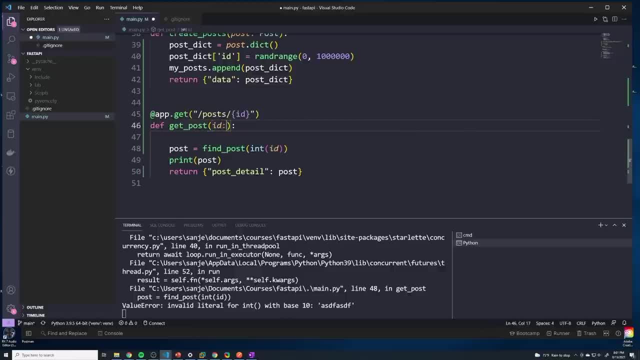 Well, we can perform validation with fast API. So here for ID, what we can do is we can say: I want this to be an integer. So what it's going to do is it's first of all going to validate that it can be converted to an integer, and then it'll automatically convert. 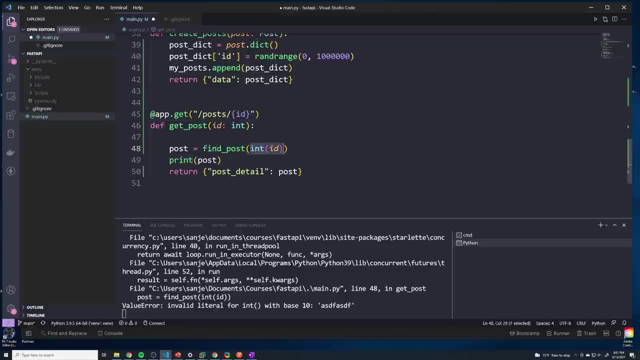 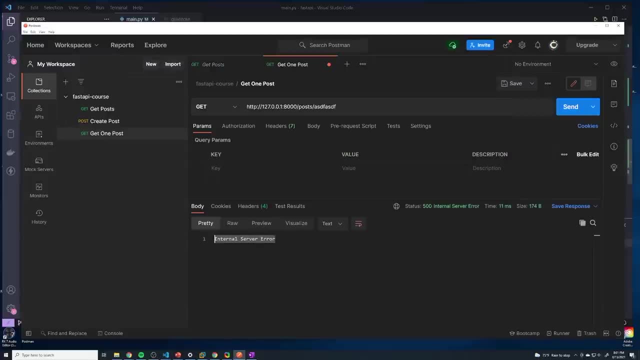 it to an integer for us, So we no longer have to convert this ourselves. So here I could just pass an ID, because this will make sure that it's already converted. And so now, if I save this and I change this back to a number, first let's make sure that everything's working. 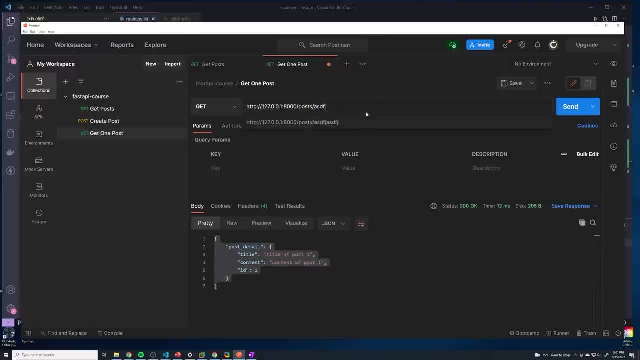 So it automatically converted it to an integer. And now if I pass in you know a string, it's now going to throw an error. it's gonna say: for a path parameter of ID, you can see that this value is not a valid integer. And so now the front end has a good way of understanding. 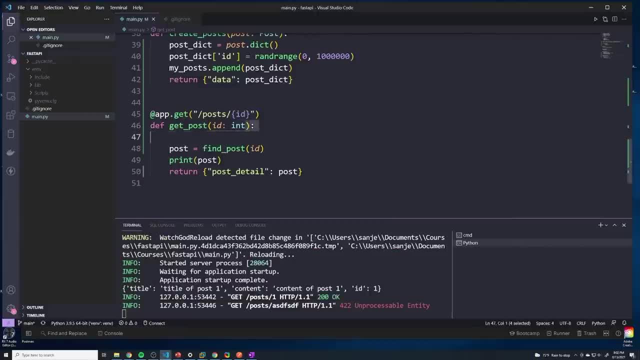 what they did wrong, And you know this can be anything, right. So if you wanted this to be a string, right, we can have this automatically get validated as a string and convert it into a string, So that if they do actually send a string, no errors, right. And then, if they, 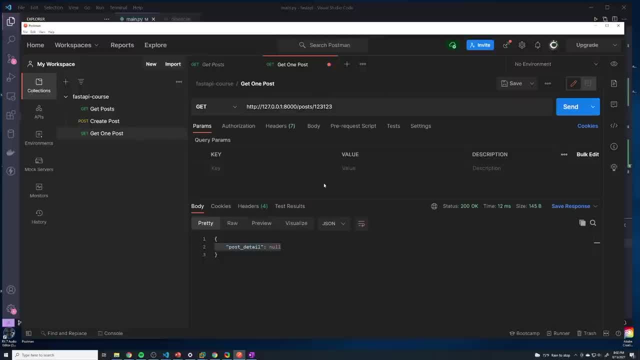 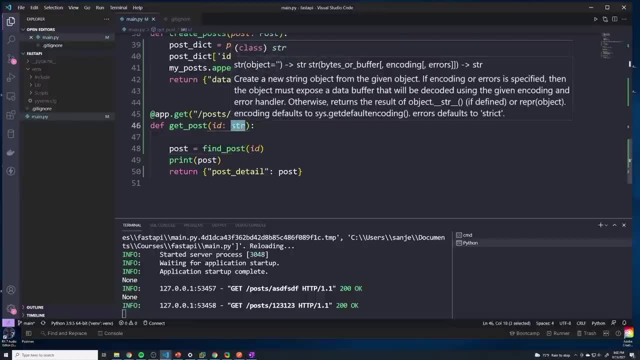 tried to. actually, even if you put in a number, it's not going to throw an error, because any number can actually be converted into a string. But we want an integer, So I'm going to change this back to an integer And then we'll just code this as to perfect. make sure you save. 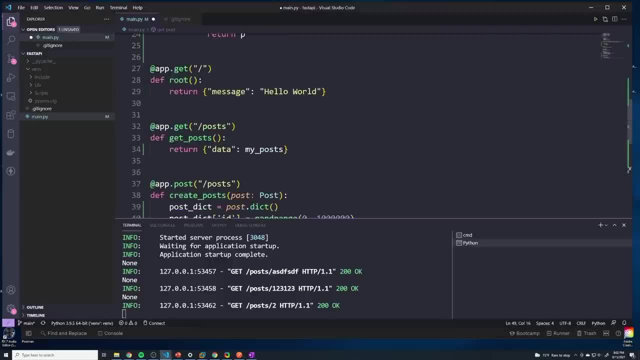 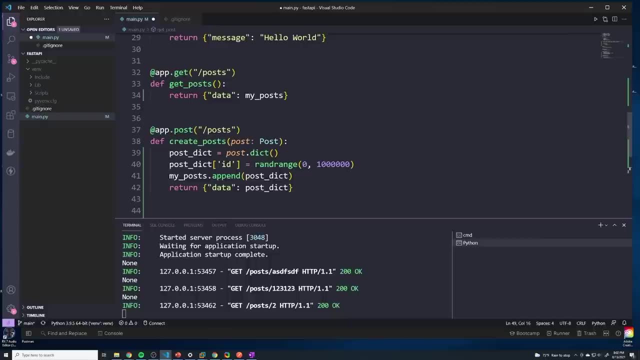 your request, And so now we've now implemented our third function within our CRUD app. So we've just got two more. we got to handle updating and deleting posts, but we've got all getting all posts: creating a post and then getting an individual post, And you'll. 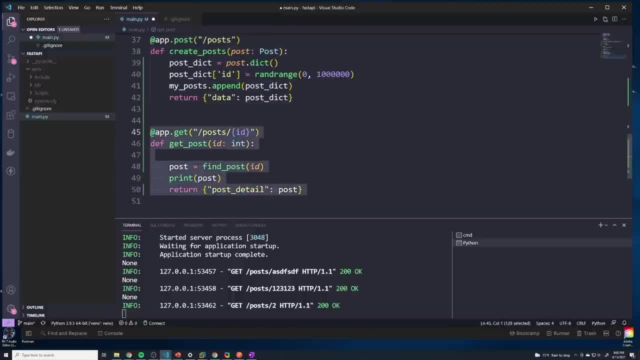 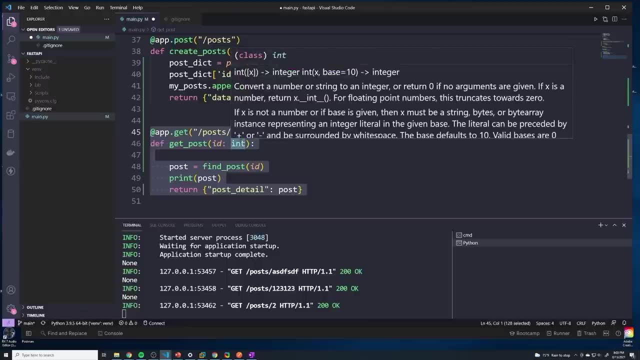 see that for the last two it's pretty much the same thing. right, we just have to define our specific decorator and then define the logic for actually creating and deleting a post from that array, or updating a post as well. Now, before we move on, I do want to. 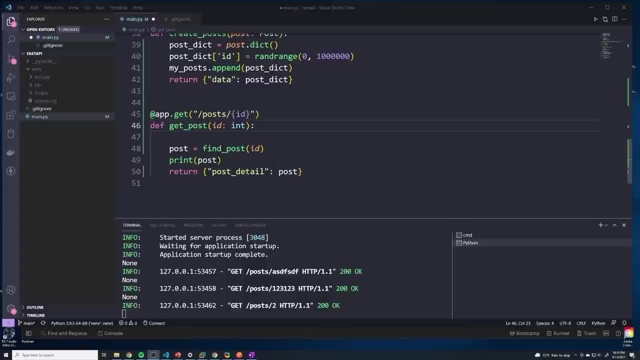 show you guys one potential issue that you can run into if you don't quite understand how these routes work and how order matters Within fast API. So what I'm going to do is I'm just going to create a dummy route And you guys don't need to follow along on. this is just a quick little demonstration And 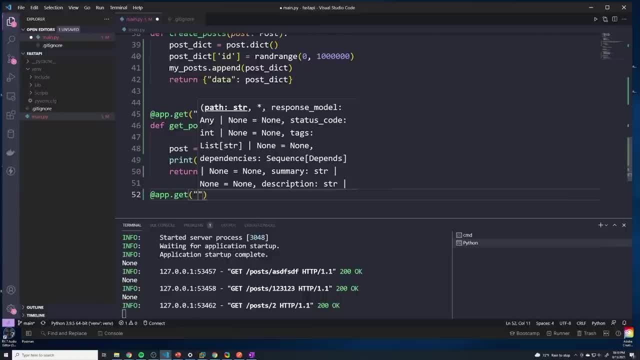 I'm just going to make this a another get request or handler for a get request, And then this one's going to be posts slash latest. So what this will do is when the user sends a request, I get requests to this specific path. I just path we're going to grab whatever. 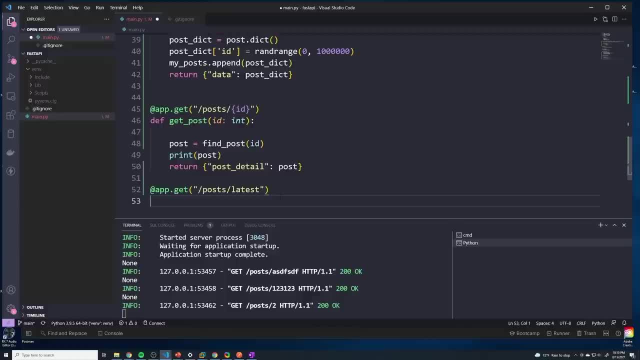 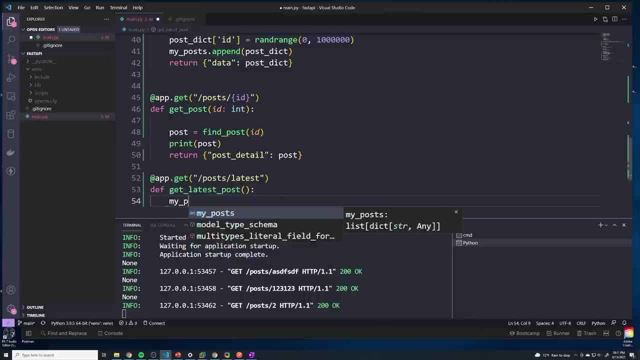 the latest post is, And so here I'll just say def, get latest post. And so all I'm going to do is I'm going to reference our my posts list And I'll say: we'll get the length of my post, And then we'll just minus one. So this will grab the 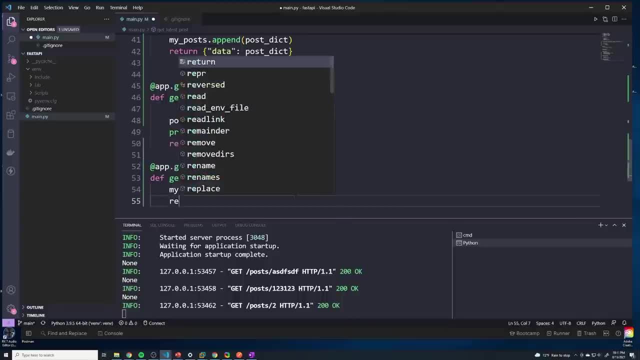 latest post, And then what we're going to do is just return that Here we'll say detail, And then we'll pass in And actually let me store this in a variable post equals, and then we'll return post, We'll. 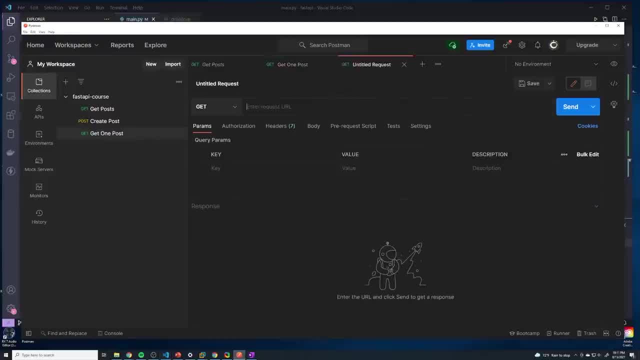 save this and I'm going to show you what happens. So let's create a new request. I just copy the URL from the previous one And here we're going to change this to latest. Let's see what happens. Interesting, we get an error. So what exactly happened? Well, let's take a look at the error. 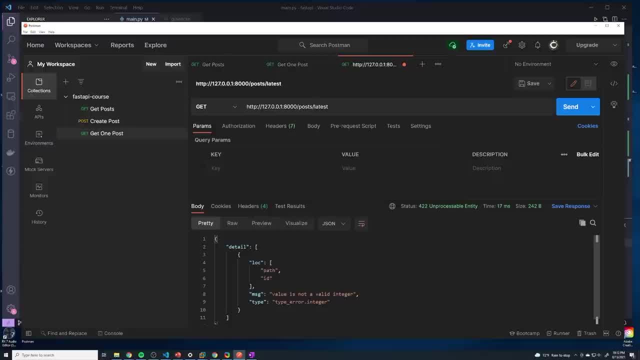 It's saying that we have a path parameter called ID, And it looks like it's saying that this is not a valid integer, So I'm not even sure why it's referencing this error. I guess, if we take a look at our code, right, there's there's no path parameter here. So what is exactly? 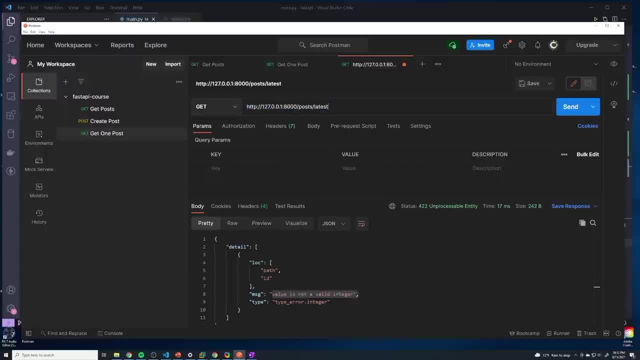 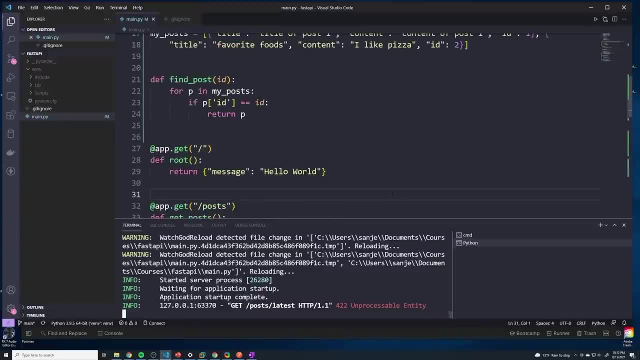 happening. Well, let's take a look right. Our request looks like this, So it's going to slash post, slash latest. So when we send this request, what's going to happen is that we're going to start all the way at the top And fast API is going to go through the list. 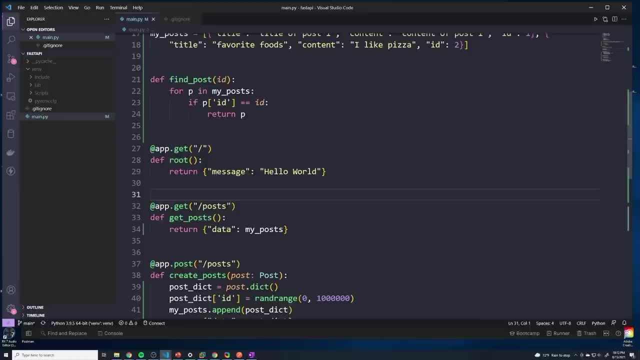 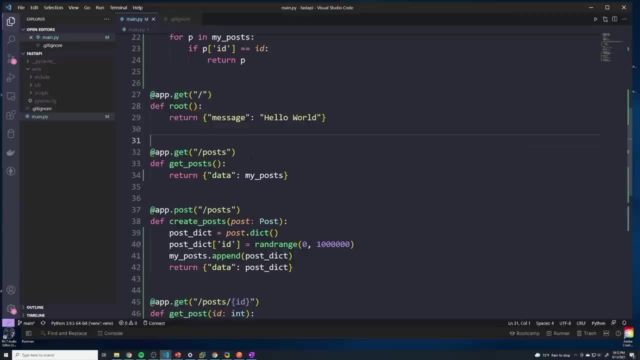 of all of our paths And it's going to find the first match. So we have one at just the root URL, So it's not going to match that. We have one at slash posts. it's, once again, not going to match. 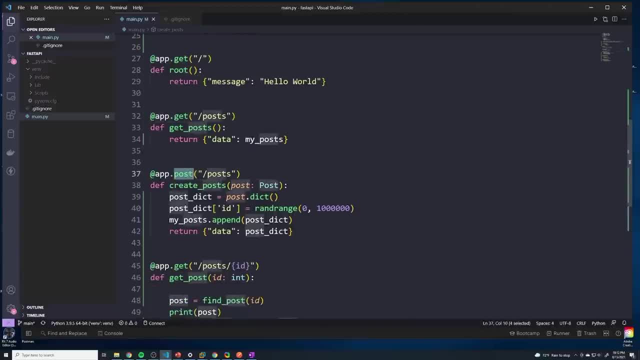 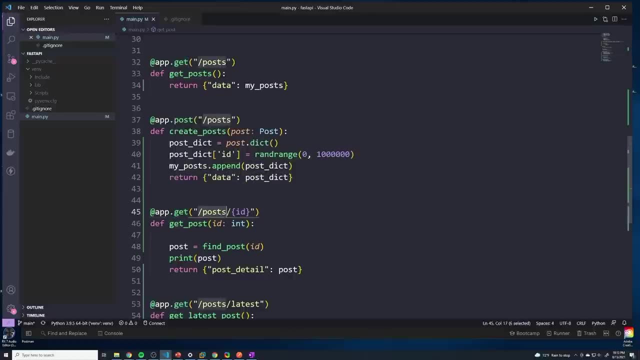 that this one is for a post request, So it's not going to match that because we sent a get request. But then something interesting happens here when we get to this get request. Right, So this is handles a get request and then it matches slash posts and then some. 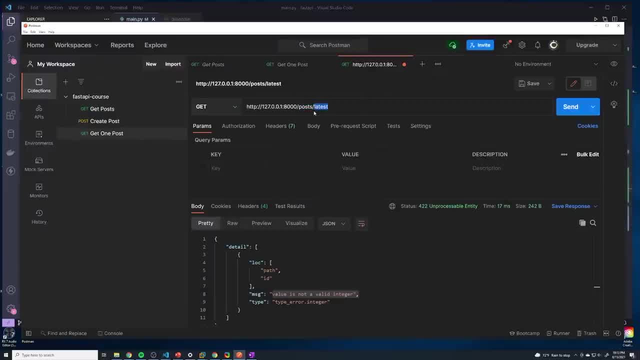 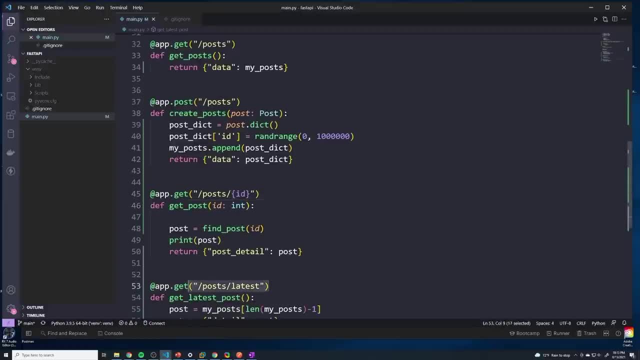 variable, So technically that variable could be latest. you see the issue that we're running. we're running into because there's no way for fast API to know that that route was meant for that, that request was meant for this specific path, right, because it does technically match. 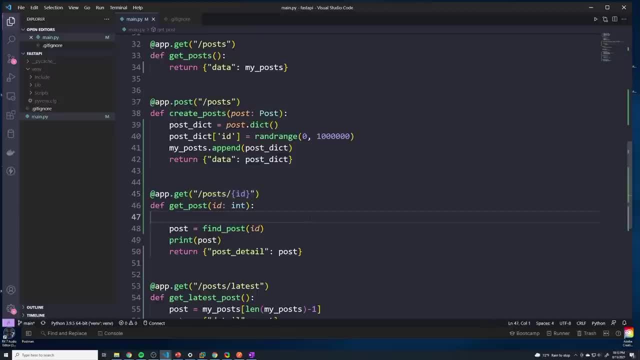 on this, And then what happens is, since it matches on this route, it then tries to perform validation on ID, which is, in this case, it's going to end up being latest, And then it's going to throw an error because latest can't be converted to an integer, And so this is. 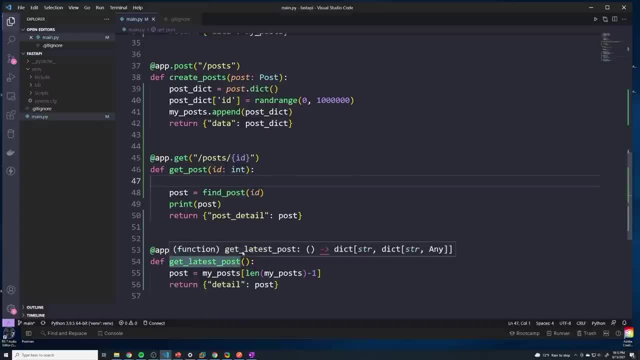 the example of where order matters. So you have to be careful when you structure your API, especially with your, with your path and your URLs. you want to make sure that you don't run into this type of issue. So you know one thing: in this case, you could do is just move this up. That would fix the issue. Because now, if 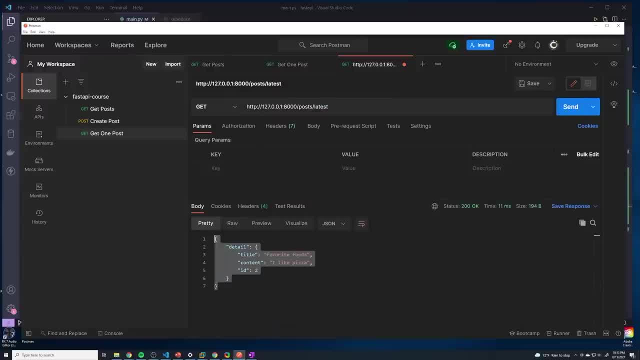 you save this and then run this, right, it works. And if you try to reference a specific ID, that's going to work as well. Well, in that case, let's try one Yep, And so that works as well. 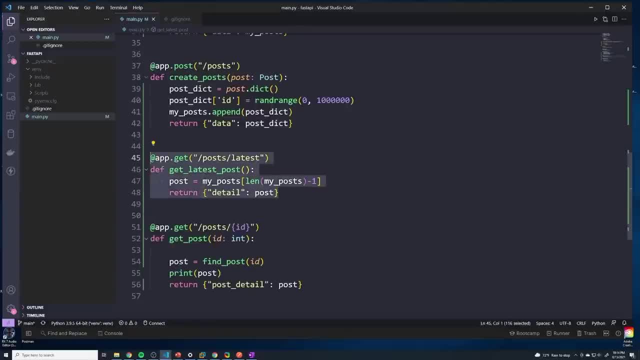 because slash post slash, one will never match this one, it'll only match this one, And so be very careful when it comes to the order. it always works top down, So anytime you're working with path parameters, it could potentially result in you guys accidentally matching other routes by 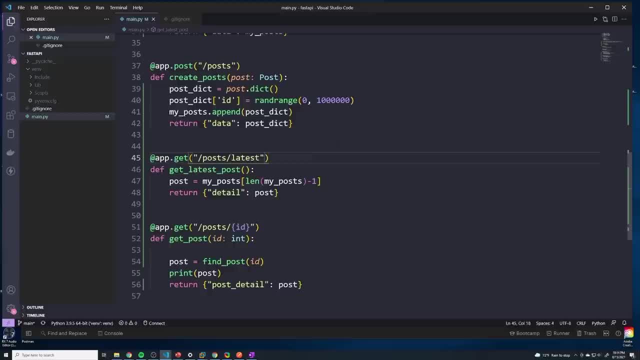 accident. So you know there's different ways to get around this. Like I said, you can just move this up. Or, if you wanted to change the URL altogether so that this is like a slash post, slash, I don't know. you know, just put in another keyword something like a recent or something. 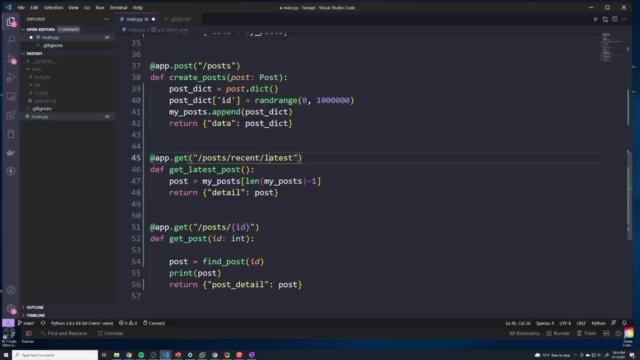 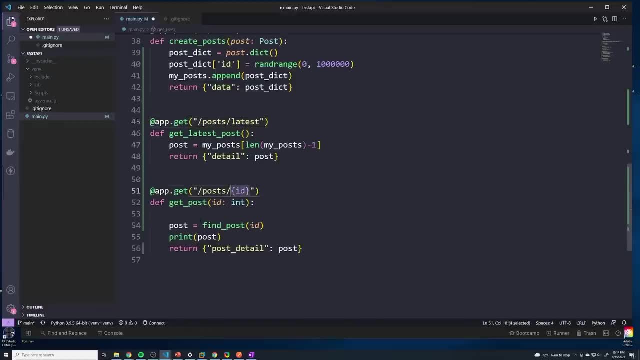 recent slash, latest or something. Well, actually, even then, that would yeah, And so just keep. And so I just want to make sure you keep that in mind when you're structuring your API, Because anytime you have a path parameter, it could result. 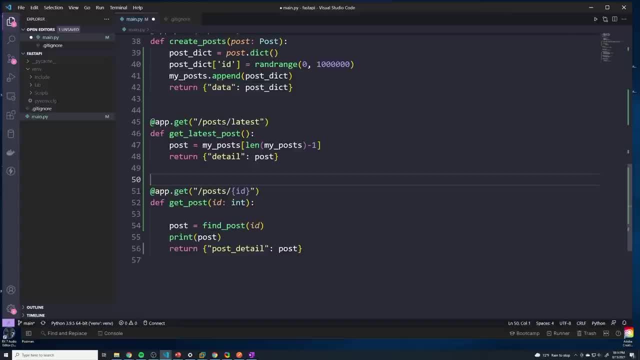 in you accidentally matching requests that were meant for a different, for a different route, So I'm just going to delete this. this was merely just for demonstration purposes And I just want to make sure that you guys understand the fast API just looks at all of your paths and just works. 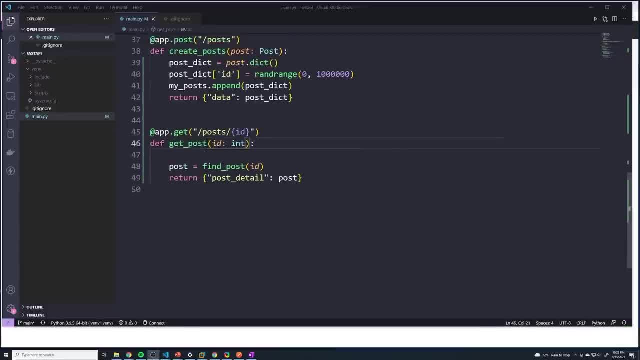 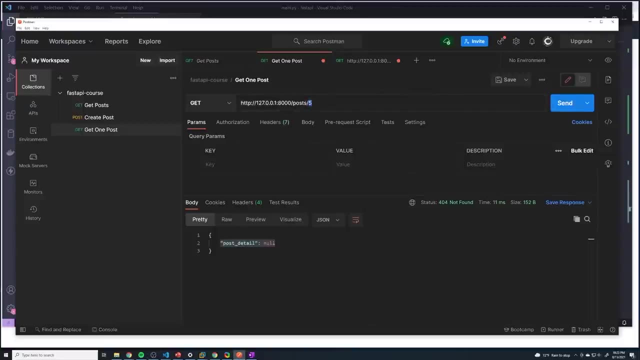 its way down the list till it finds the first match. And then you can see here, if we go back and we go to our post man real quick and we do get post path operation, specifically the one where we retrieve one specific post, we do run into a little bit of an issue. So if we go to our post man real quick and send a request to get one post, but in this case, instead of doing one or two, what I want to do is I want you to put in the ID, put in an ID that doesn't exist. So we only have right now posts with an ID of one and two. what happens if we send it with a ID of five? you can see what we get back. it says null right. So we have to get rid of that one and we'll get rid of that one. And if we send it with an ID of two, we get rid of that one. And if we send it with an ID of three, we get rid of that one. And if we send it with an ID of four, we get rid of that. 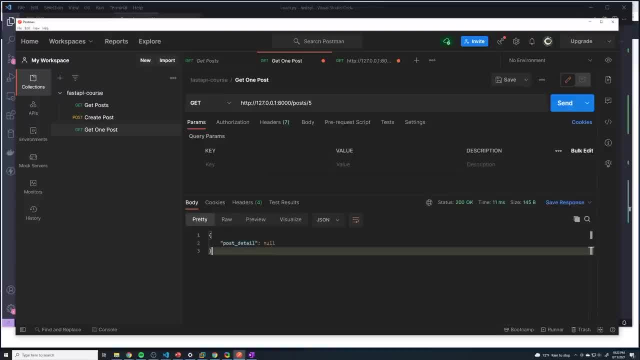 right, And I don't like that because it doesn't really give the front end any feedback as to what exactly is happening. So they don't actually know. you know, they don't know if some kind of error occurred or if we were unable to retrieve this information properly, or if there's 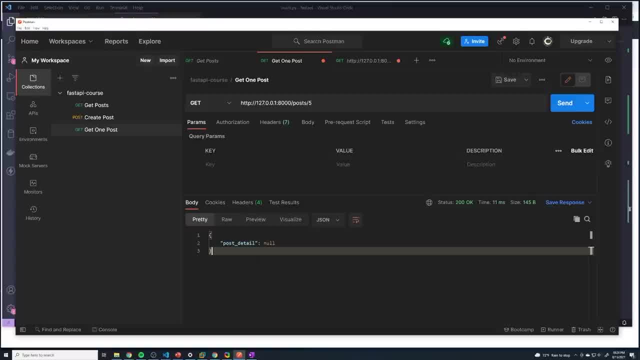 a server error or if this item doesn't ultimately exist, And so we need a way to accurately tell the front end that, hey, the ID that you're searching for does not actually exist in our database, And the best way to do that is through a method that I'm sure you guys are already a little bit. 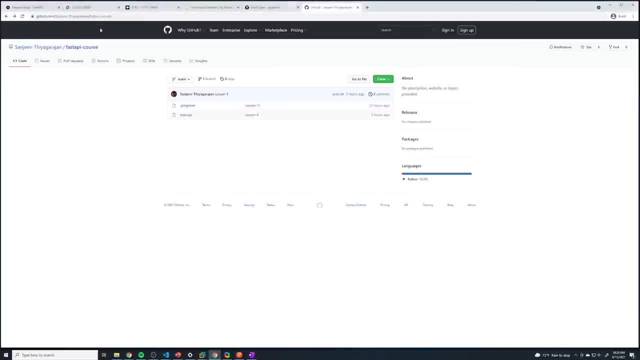 familiar with. So right here I've got my GitHub page for our course And you can see it's just GitHub, my username and then the name of the repo. But if I search for, if I put in a whole bunch of letters afterward, what's going to happen is GitHub is going to look for a repo with this. 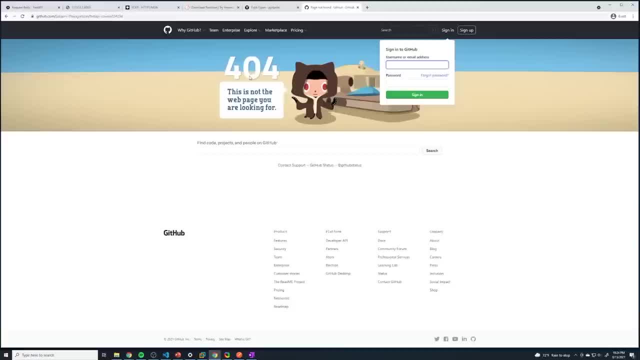 name that doesn't exist And let's see what happens. It gets a 404.. And I'm sure you guys have seen a 404 error at least once before in your life. So that's a specific HTTP status code that represents that this item was not found, though it does not exist. 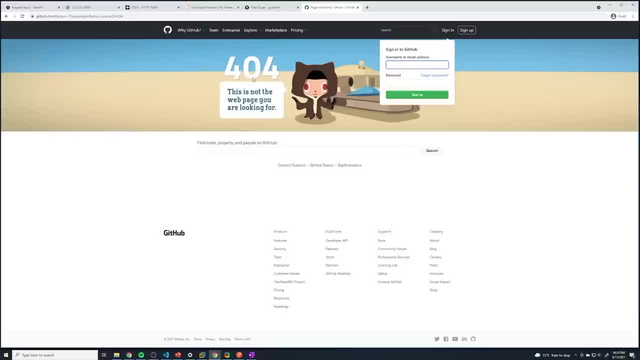 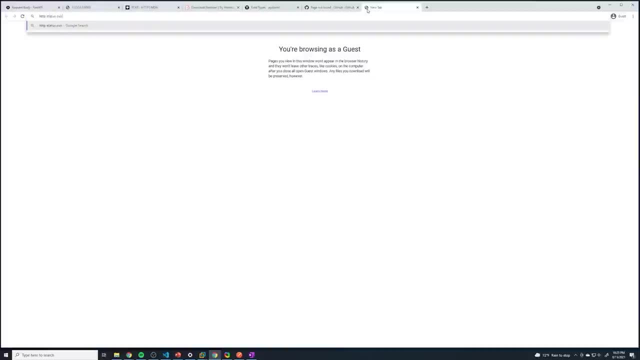 And HTTP status codes are important. We haven't really talked about it in this course up to this point, But there's a lot of different status codes And if you actually just search for HTTP status code, you can just grab one of the top links. I'm going to go take a look at the Mozilla one. 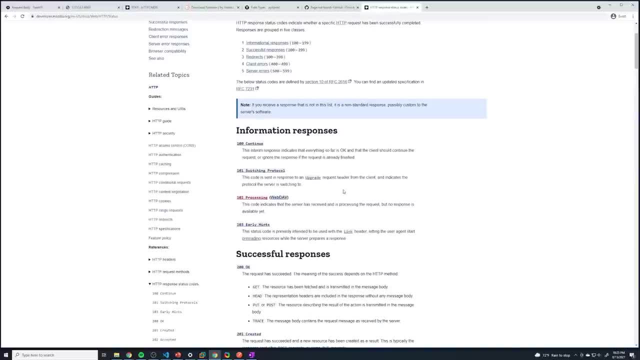 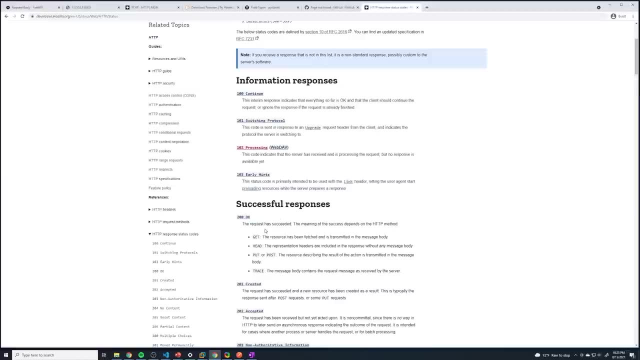 and you'll see all of the different HTTP status codes And you'll see when to use them. Now, most of the time, you're going to see that we get a 200 response back. that's the default one the fast API sends. that usually means that everything's good, everything worked, That's. 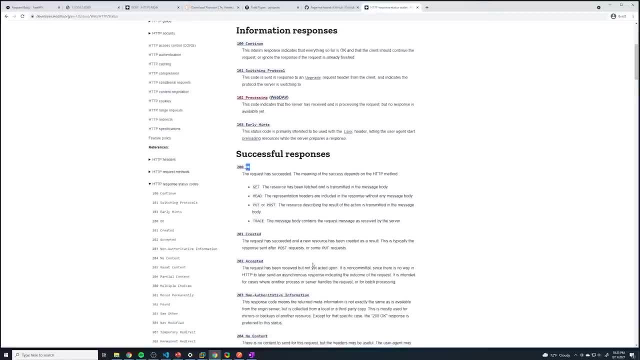 why it says okay. However, we do have other ones that we do also commonly use. So anytime you create something, so within your CRUD application for create, anytime you send a post request, usually after you create the entity, you send a 201 back instead of a traditional 200.. So there's a lot of HTTP. 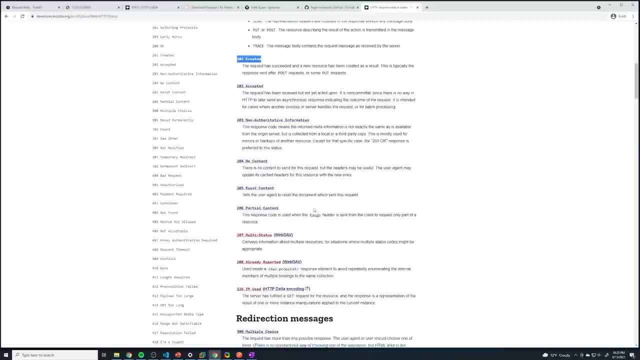 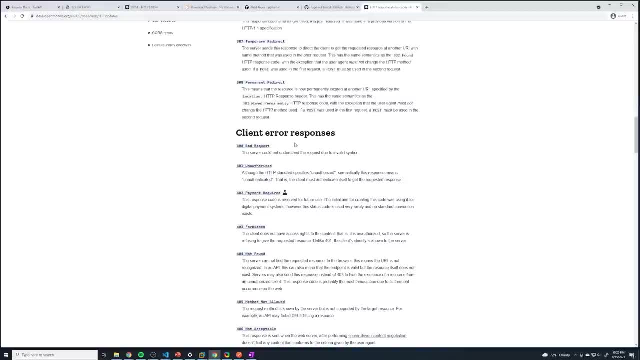 status codes And we're going to cover all of those in future lectures. But the ones we're interested in is for when we have an error. So we scroll down. 400 usually means there's some kind of bad error, something happened And, most importantly, we want the 404 not found, So the 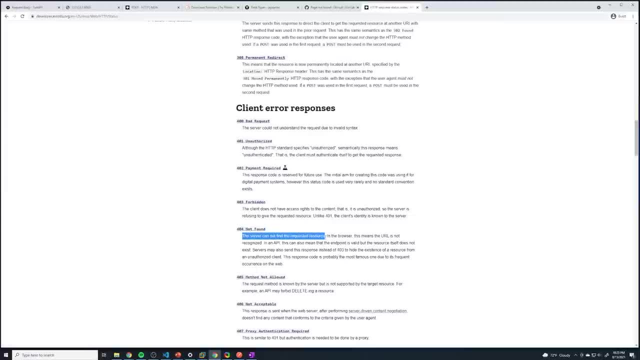 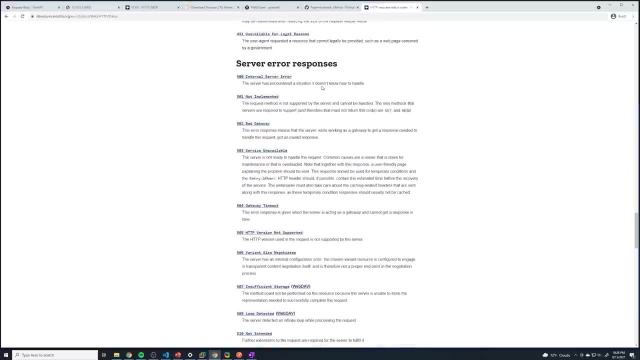 server cannot find the requested resource. So that's exactly what we're looking for. Keep in mind, there's also 500 status codes, which means you know some kind of server error, server error or server failure. So we're going to do is- I'm going to go back to our code, And what we need to do is we need to. 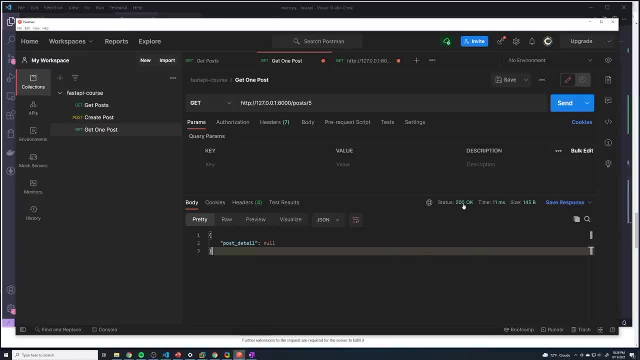 manipulate the response, Because right now we're getting a 200.. Back we're getting a status code of 200.. If I send it, it says null, and then it just sends 200.. So that doesn't really give us a. 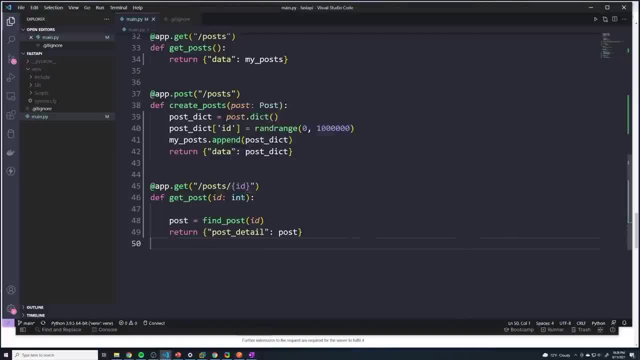 good idea as to what's happening. So how do we manipulate the response? Well, we have, you know, have to first of all import the response from fast API, And then what we're going to do is we're just going to pass it in as a parameter into our path operation function. So I'll just call this: 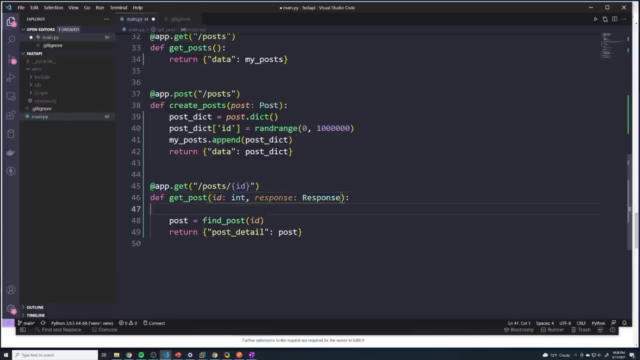 stored in a variable called response, And so once you get access to the response object, we can tweak it however we want. So what I'm going to do is, after we search for post, if we didn't find a post, I'm just going to do a quick check. I'm going to say: if not post, right, that means, if we didn't. 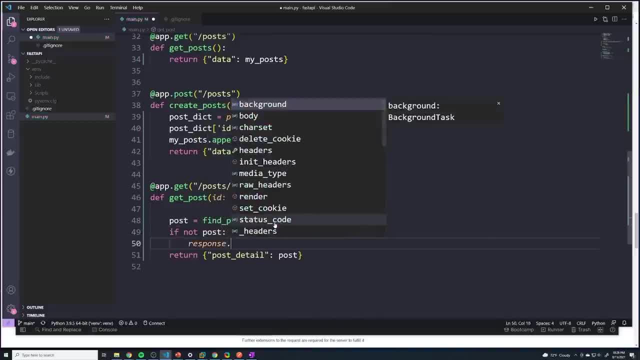 find a post. what we're going to do is we're going to set the response And then we're going to grab a property of a response called status code. So here we can tweak the status code of the response. I'm gonna say, Hey, I want this to be a 404.. All right, now let's save it. Now, if I hit send. 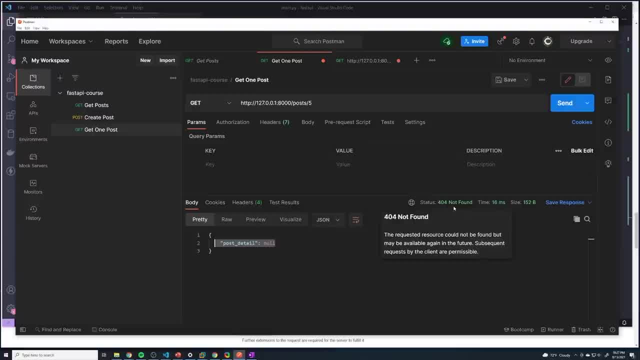 it still says post detail none. but take a look at the status code. it's now updated to 404.. And if I change this to an ID that does exist, right, we get the post properly and the status code changes to 200, which means everything is good. 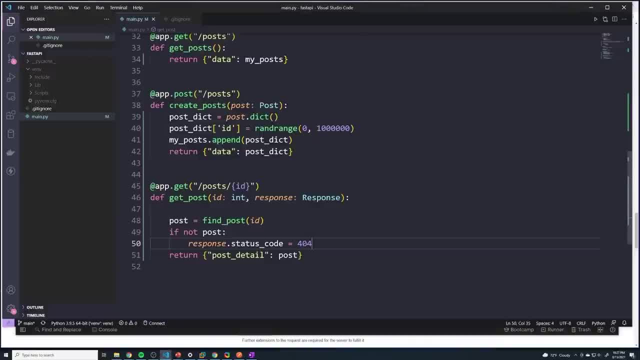 That's one way of doing it. However, there's a slightly better way of doing it: Same concept, But instead of hard coding the value or trying to remember it, what we can do is we can import from the fast API library something called status. 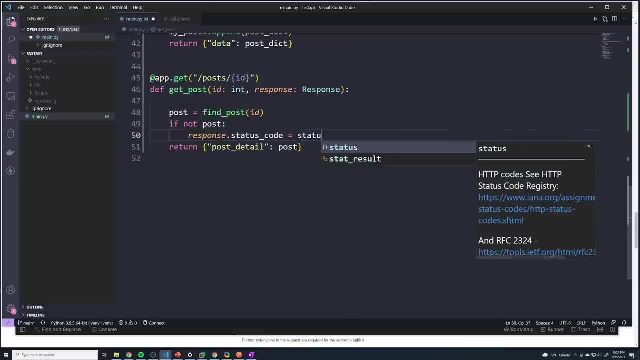 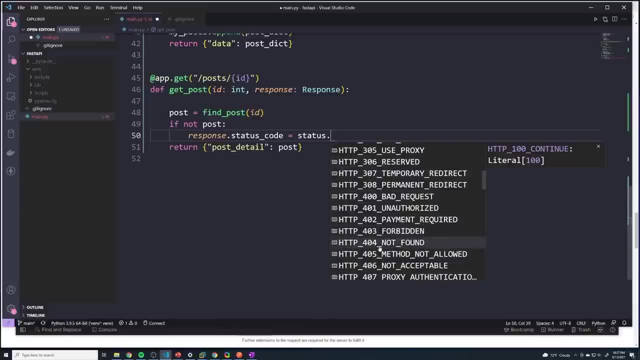 And so now, instead of having to remember what to use, we can just type in status And then it's going to show you all of the different HTTP codes. And so now you can do that And you can just quickly just look through which one- ever one- sounds the most accurate. 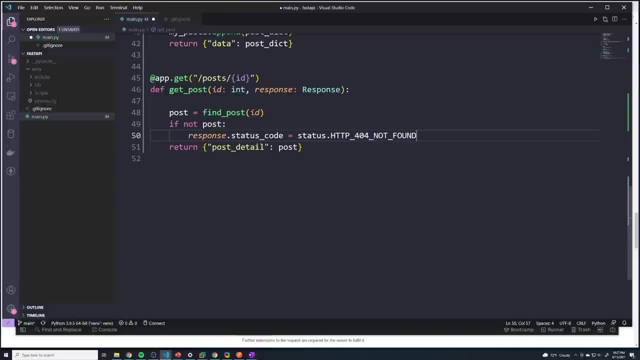 So we'll grab the 404.. And now you don't need to worry about putting hard coding in a number we can just reference. You know, I guess it's an, it's probably an enumerator, but I'm not really sure. So it doesn't really matter. And then that's all you have to do. So let's test this out again. 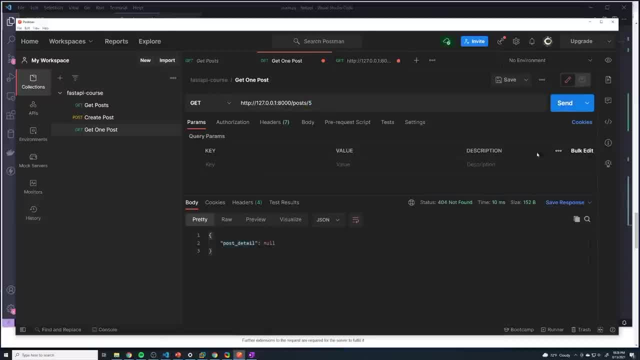 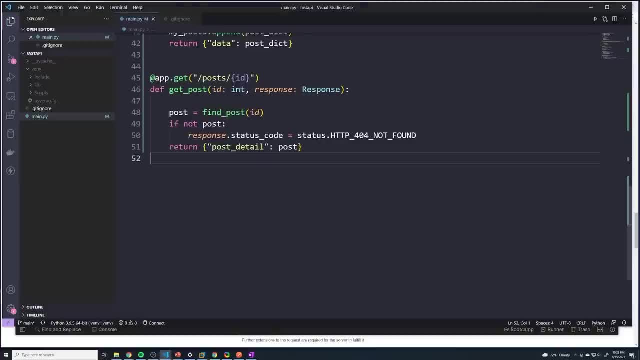 So 200 good changes to five, 404.. Perfect. But the next thing I want to do is I don't want to return. that looks ugly, So instead I'd like to actually throw an error. So in this case, in this if statement, I'm just going to call a return. that only is going to ever. 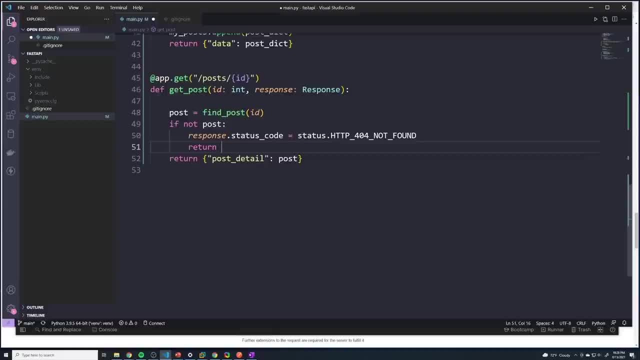 run if post doesn't exist And we'll just say, in this case, detail, or we'll say message. I'll just say message f, string. I'll say post with ID And we'll pass in what was the ID. I'll. 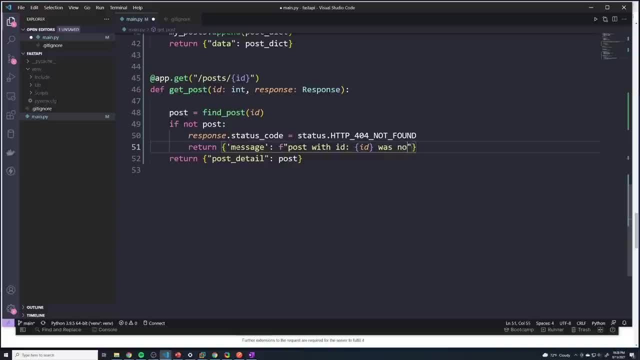 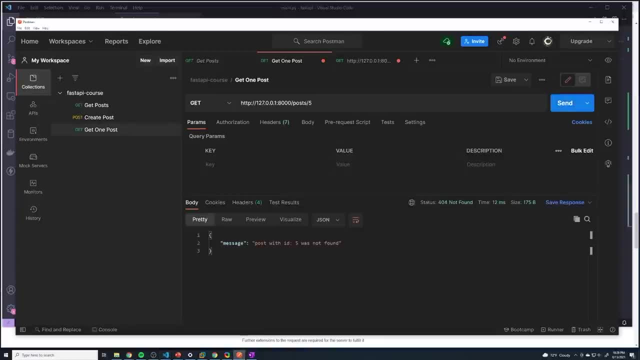 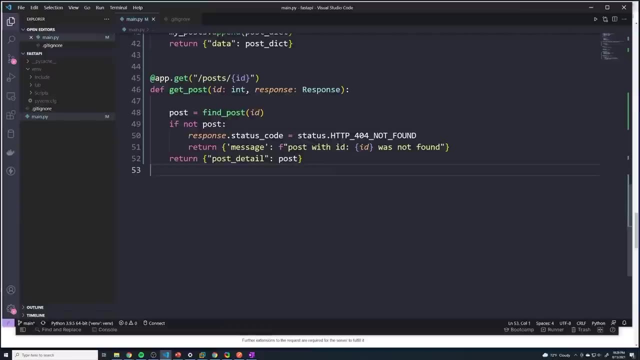 say was not found, All right. and now, if we try this, okay that we get our air post with ID was not found And that matches up with the ID that we gave it And we got our 404.. Now, this was a. this is one solution. However, I think this is a little. 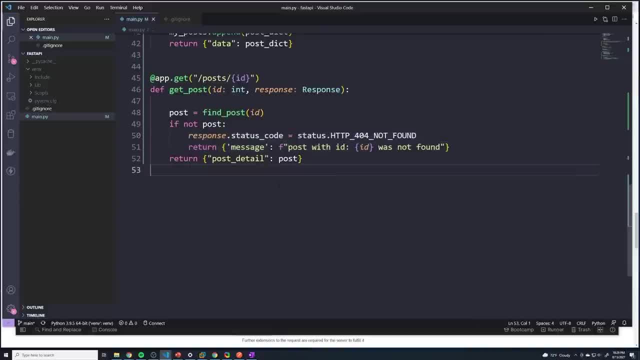 bit sloppy And there's a better way of doing it. Instead, what we can do is we can rage raise an HTTP exception. So this is a built in exception into fast API that will automatically you know you can pass in what the 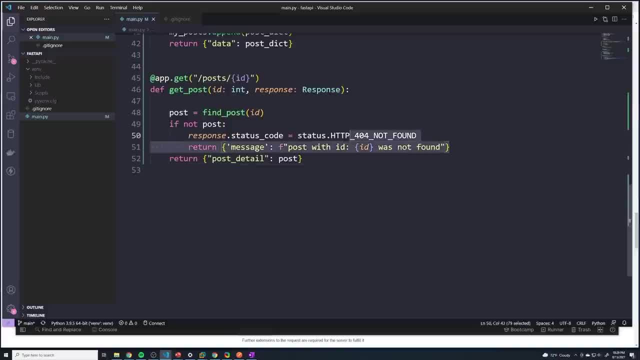 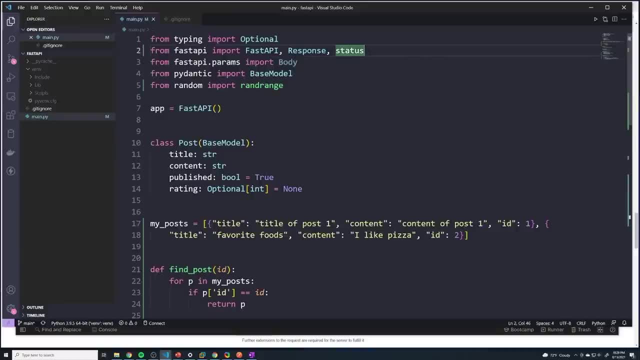 specific error code you want, as well as the message, And so that way you don't have to hard code all of this, And it just makes everything look a lot simpler. So we'll go to the fast API up here And we're going to import something called HTTP exception, And now we can. 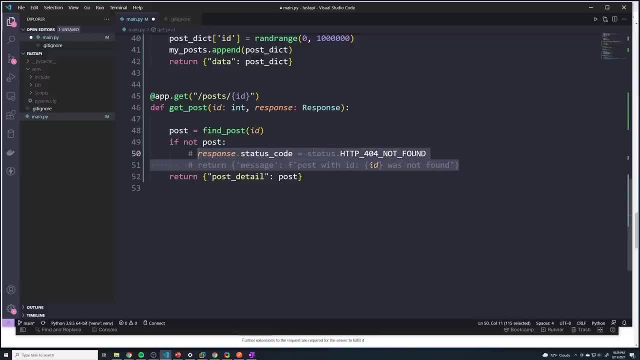 delete all of this nonsense code. Actually, I'm just going to comment it for now, just so I can reference it in a second- And all we have to say is: we'll raise an exception. So we raise HTTP exception, And then we have to pass in two things. 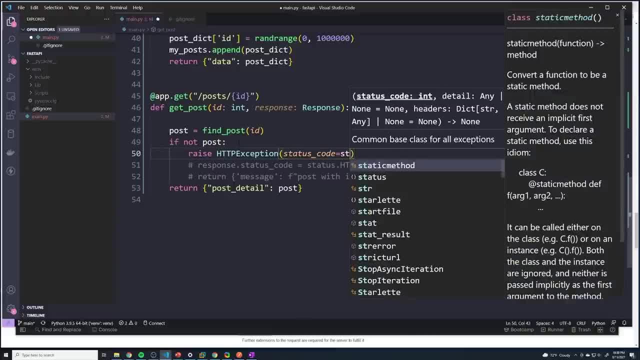 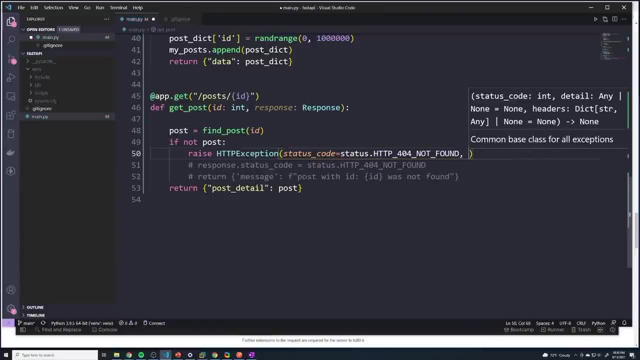 So first is the status code, So we'll set the status code to be status, And then same thing, right? So far nothing's really changed. And then here we'll just pass in the value for detail, which is going to be the message that. 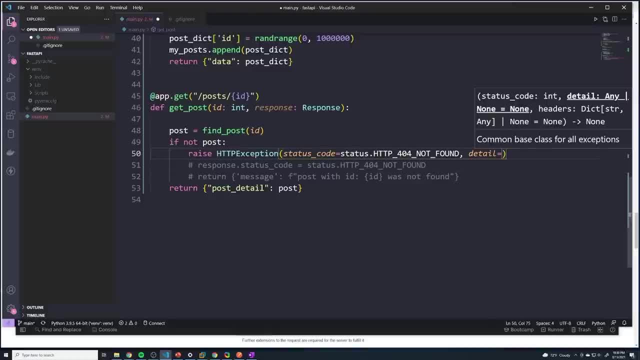 fast API automatically responds back with- and I'm going to pass in the same exact F string, And so now we've basically replaced this with just this one line right here, this HTTP exception. I think this looks a little bit nicer. I don't like having to do the set the. 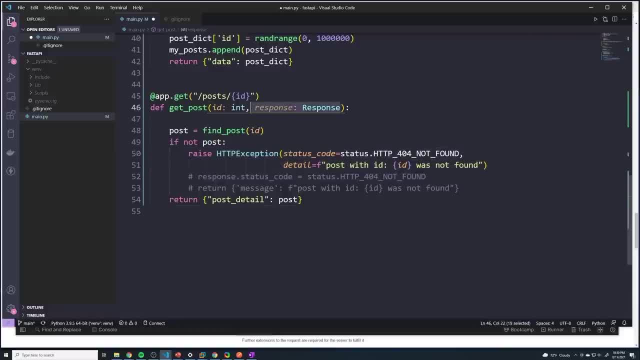 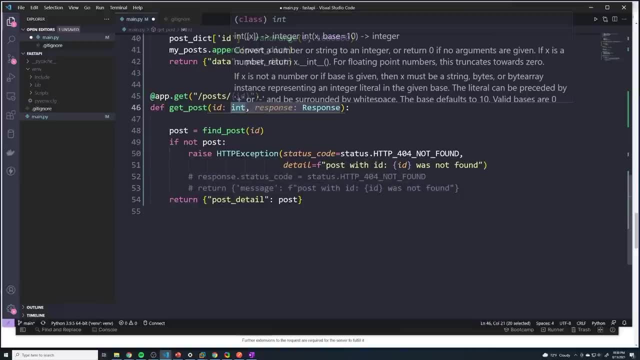 response and then having to pass in. I don't like having to pass in the response into the path operation function, having to set a property and then having to return my message. we can remove all of this nonsense And I can get rid of all of these comments, And I think this is just a little. 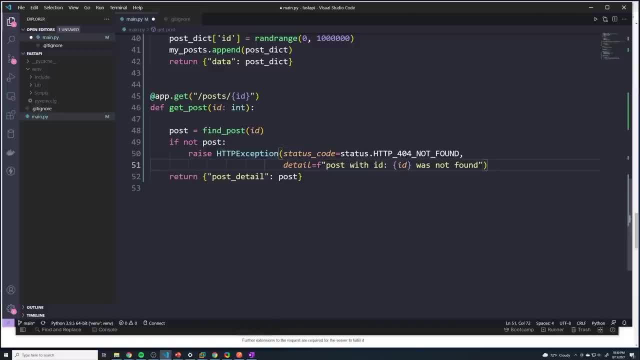 bit cleaner And moving forward. we're going to be using these HTTP exceptions a lot, Because all we have to do is just pass in what's the HTTP status code and then the message we want to send back to the user, And then that's what's going to be sent to them. So now, once again, we're going to try this. 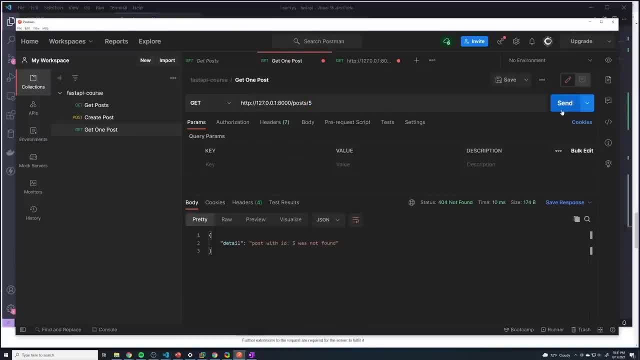 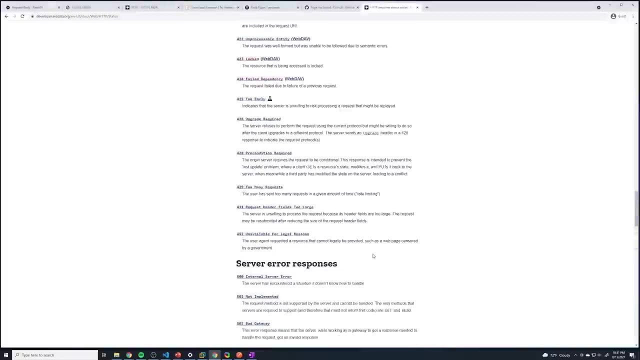 out And look at that Right. so we got the 404.. And we got the message, the detailed message, right, lot cleaner, a lot simpler. Now, before we move any further and before we wrap up this video, I did mention that anytime we create something, we should send back a 201.. So if we go back to our 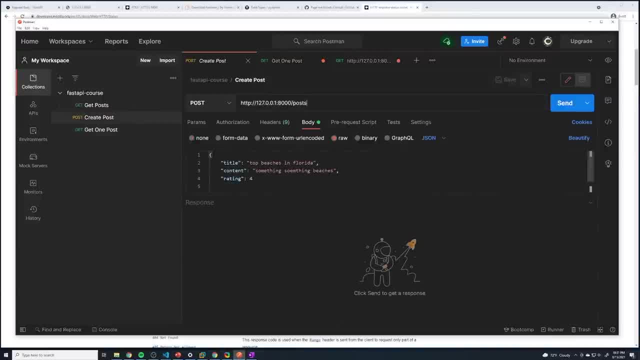 create post and then we'll just create a new post again. you just send this. we created a new post. look at the status code. that gets sent back. it's got. it gets sent back at 200.. And that is wrong. Remember anytime. 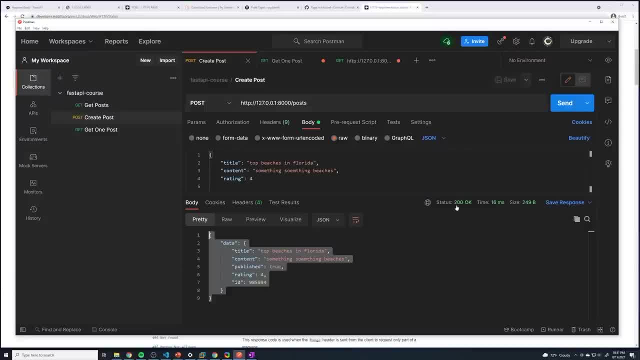 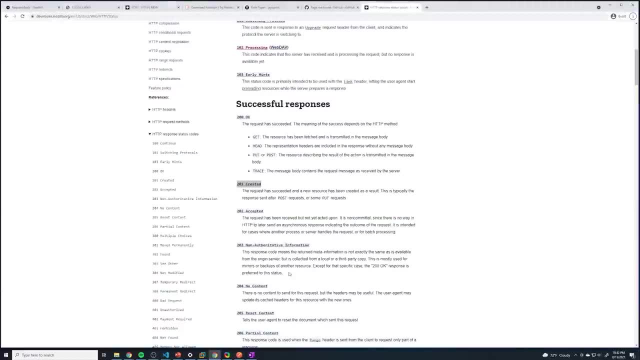 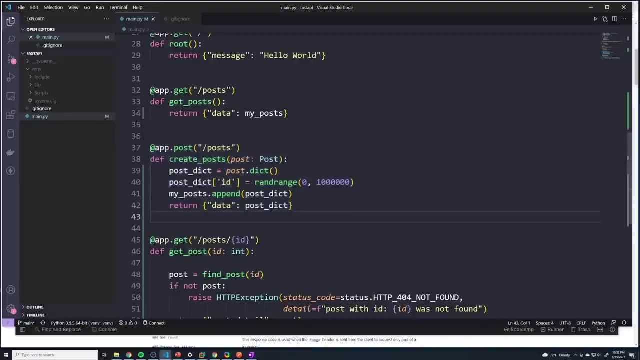 we create an entity based off of that documentation, we should send a 201.. So how exactly do we send? how do we change what the default status code is for a specific path operation? Well, what we can do is we'll go back to our code And let's find our create post And if you want to change the 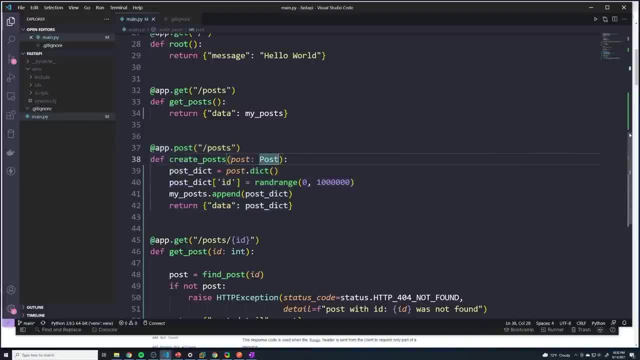 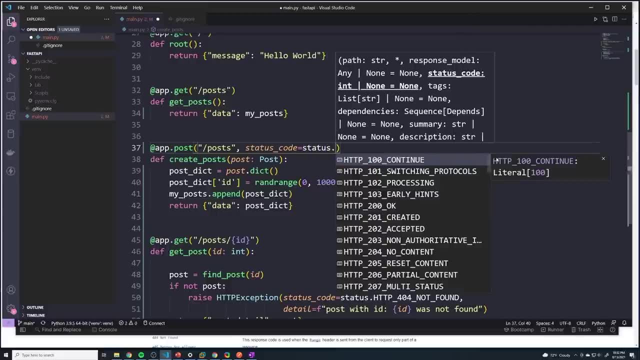 default status code. what we do is inside the, inside the decorator, we'll pass in a another option. So we'll say status code here, And then we set this to be status, and then whatever our specific status code is- so I want to a one- And then that's all you have to do. So now, 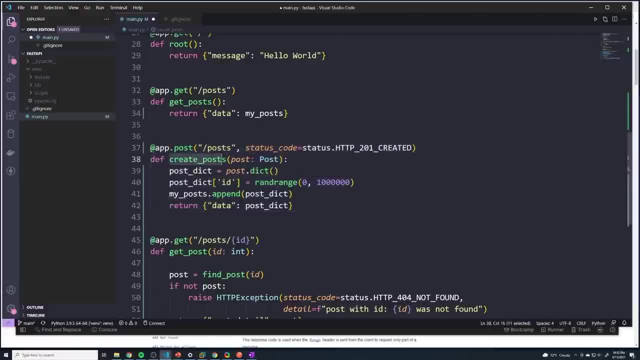 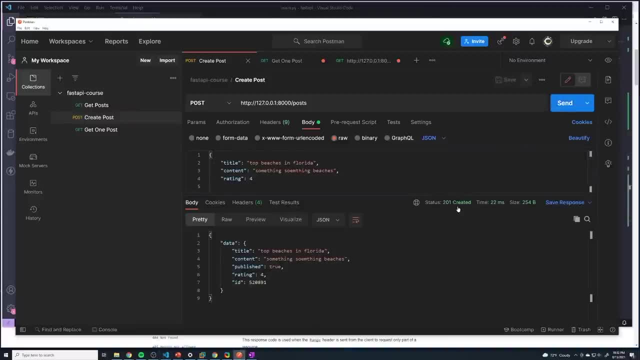 by default anytime someone sends a request to create posts. we're going to send a 201 created, So we'll save that. we'll give it another shot. If I try this again now. we get a 201. Perfect, But at this point I think you guys will have a solid understanding of how to change status codes. 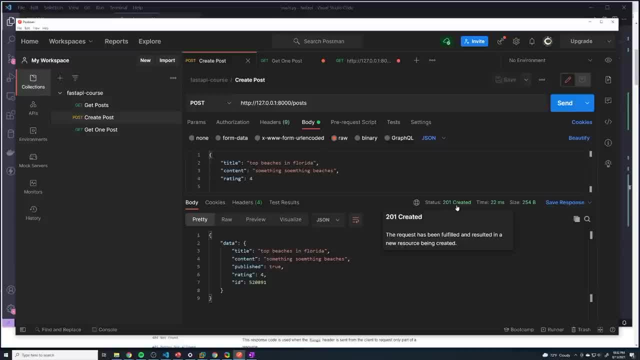 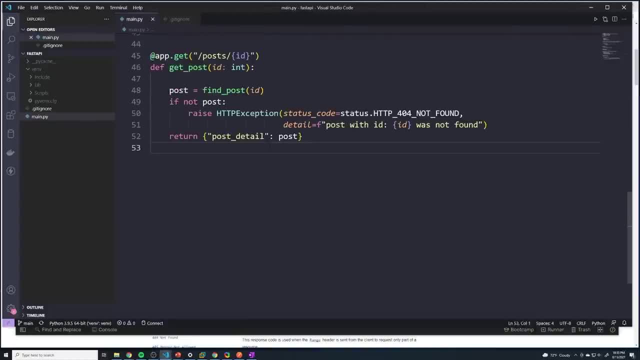 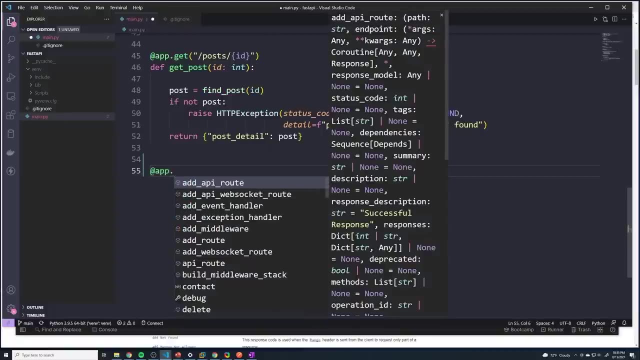 whether it's because we're trying to throw an exception or if we want to just change the default code of a specific path operation. All right, guys. so now it's time to move on to deleting a post. So to delete a post, remember we're gonna start off with our decorator And it's going to 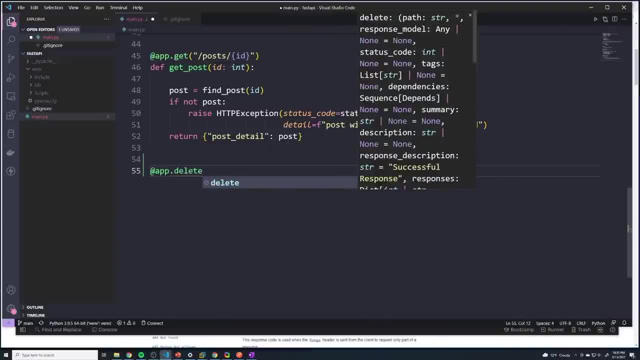 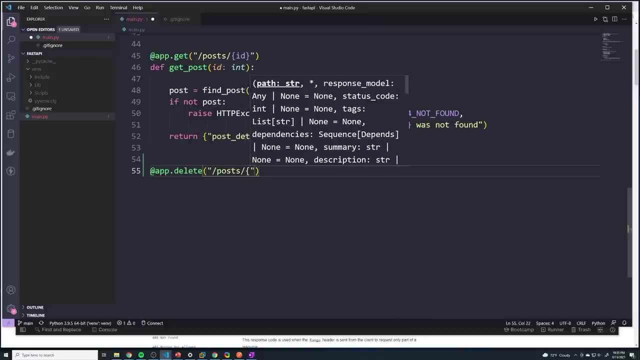 request, or it's going to require a delete HTTP request, Right, and then the URL is going to be the same, So it's going to be posts, and then we're going to need the ID So we can figure out which post to actually delete. Right, then let's define our function. 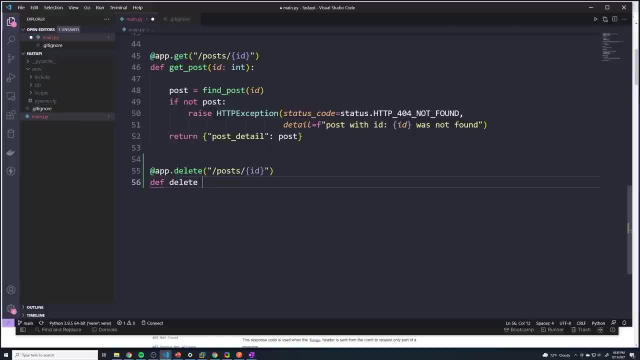 So I'm just going to call this delete post. And so here we have to implement the logic for deleting posts. So what are we going to do? Well, for me, there's many different ways. you know, deleting a post is just a matter of. 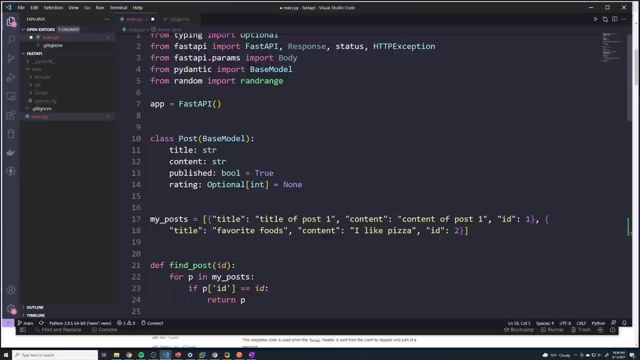 trying to figure out which specific dictionary within this array has a specific ID of whatever ID we give it, and then we just remove it from the array. So however you want to do it, go ahead and do it. I'm going to just show you the first way that I thought of. 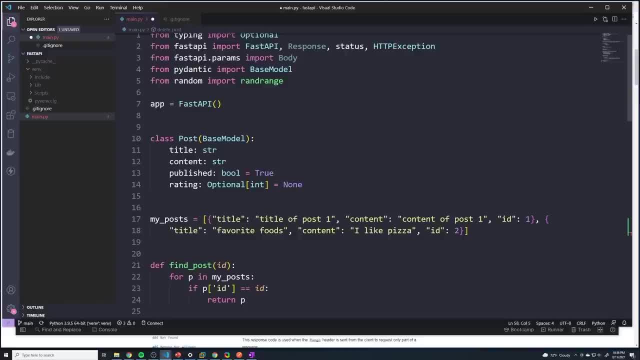 Like I said, this doesn't actually have anything to do with fast API. This is more of just simply working with Python. So I'm telling you right up front, this may not be the most efficient way to do it But, like I said, we're eventually going to implement a real database, So it doesn't. 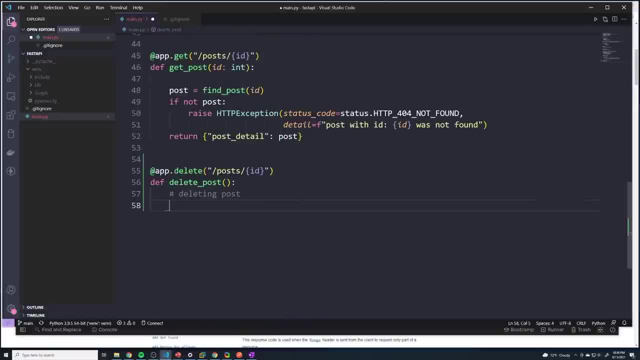 really matter how you do it, as long as it works, And so the first thing that we're going to do is I'm going to look and to find the index in the array that has required ID. we're going to look for what we're going to try to get. 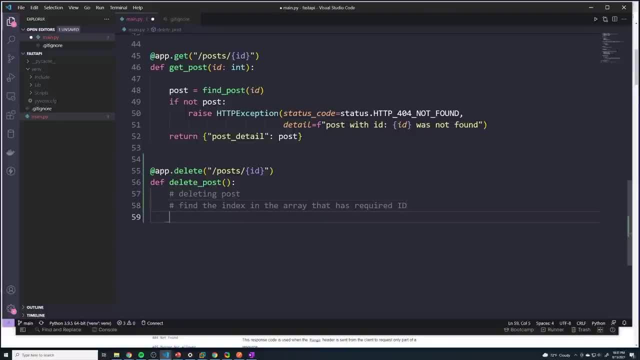 the index of that specific item, And then all we're going to do is we'll do a my underscore, posts dot, pop, and then just pass in the index, And so that's how we remove it from that array. Pretty simple. And what I'm going to do is I'm going to actually just define a function out here. 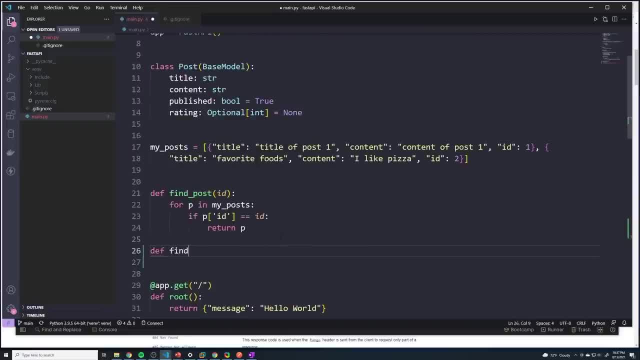 just to keep things simple. So this is going to be called find, index underscore index underscore post, And then we're going to pass in the ID that we're interested in, And then we're going to iterate over the array, But we're also going to grab. 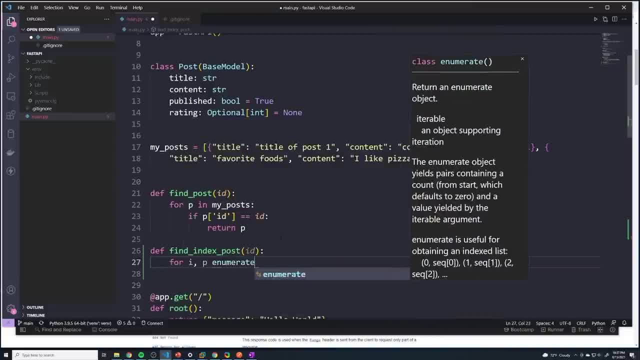 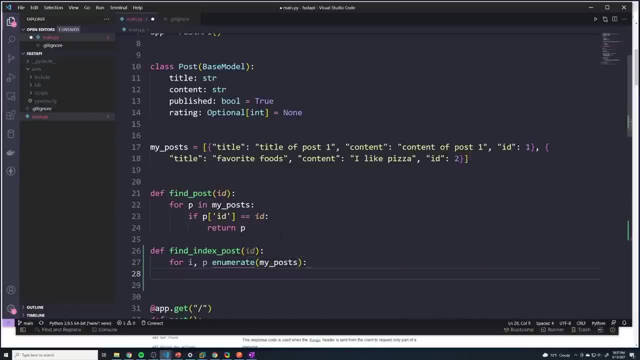 the specific index as we iterate over it- And so you do that by using enumerate, So this is going to iterate over it- we'll get the access to the individual post that we're iterating over, as well as the index, And so we'll say: if p, if the ID. 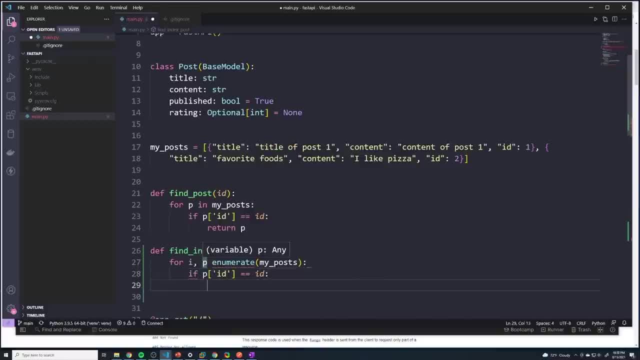 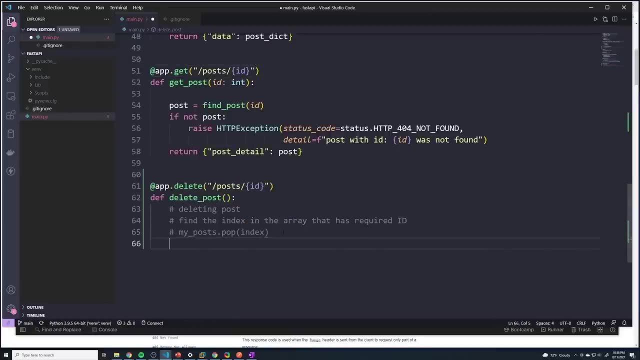 equals, equals ID. and I forgot the N keyword. here we'll just return I. so this is going to give us the index of the dictionary with that specific ID. So here we can just call that function and we'll set it equal to the index. So index equals. 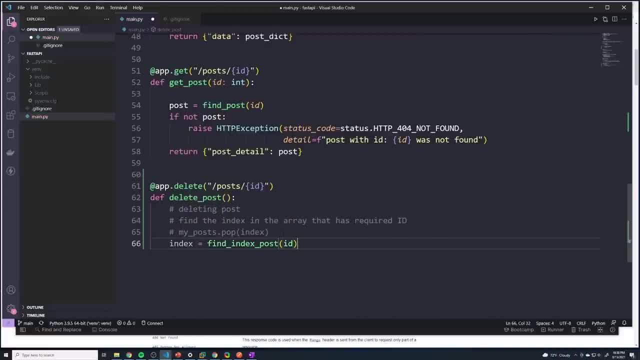 find underscore: index of post. pass in ID. So we now have the index And at this point I can just do a my post. I can copy what I just did and I can just create a code here So I can just type the. 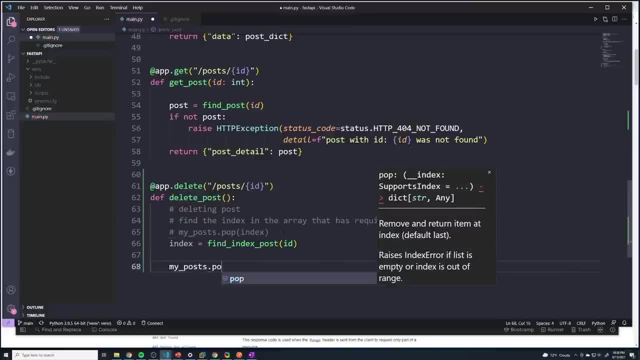 index of the post, pass in ID. So we now have the index And at this point I can just do a my post, postspop, and then just pass in index And then we'll try to do a return And then here. 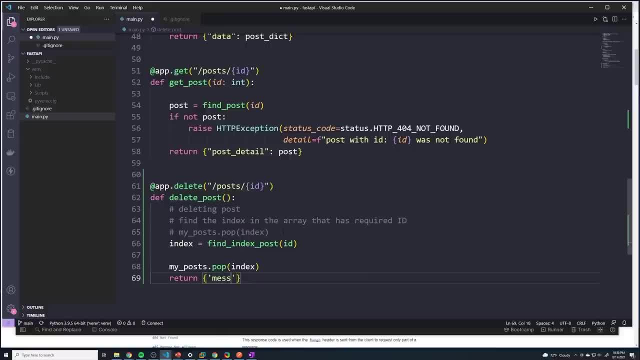 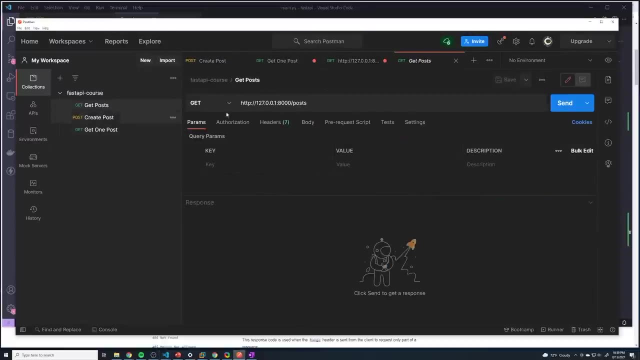 I'm just going to pass in. we'll say message, We'll say post was successfully deleted. But let's give this a shot. So, first of all, let's get all the posts. If I do a get all posts, you'll see that we have two posts And then I'm going to create a new request And this: 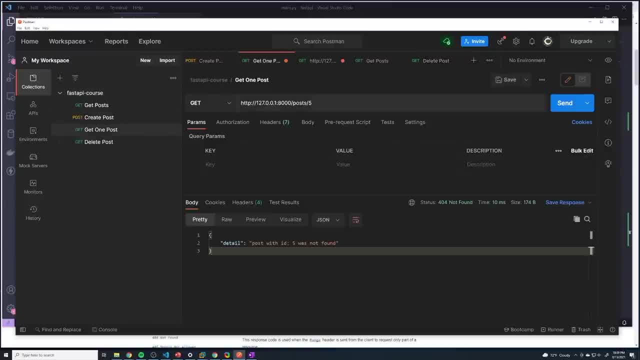 will be called delete post. Copy that URL, pass it in there. And so here I'm going to try and delete with a post of a value of one, And I realized I still have to ask get. so we're going to change the delete Right. And so now it throws an error. So what exactly? 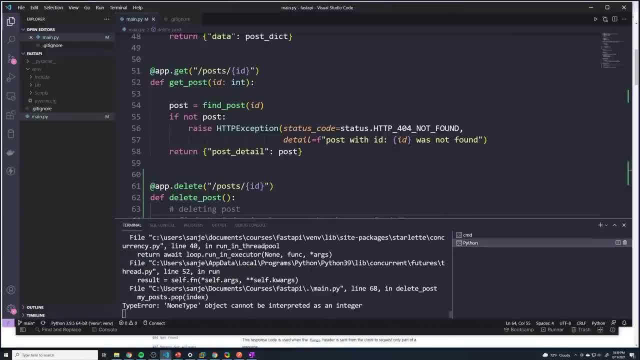 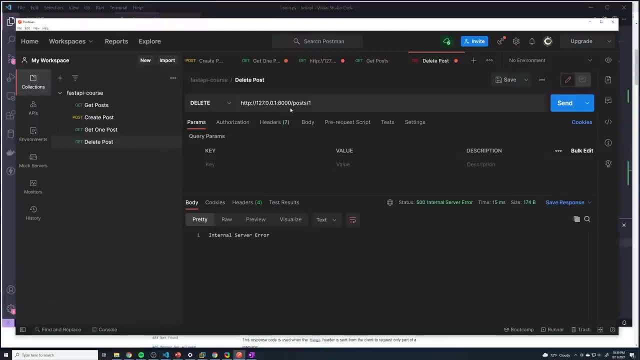 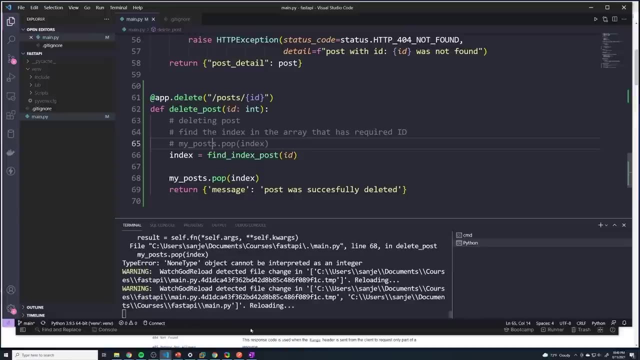 happened. Well, if we go back to here and then go back to our console, it says: says none type object cannot be interpreted as an integer. And, and I realized I forgot to actually pass in ID into our function, So that's why he was giving us that error. So now let's try this. 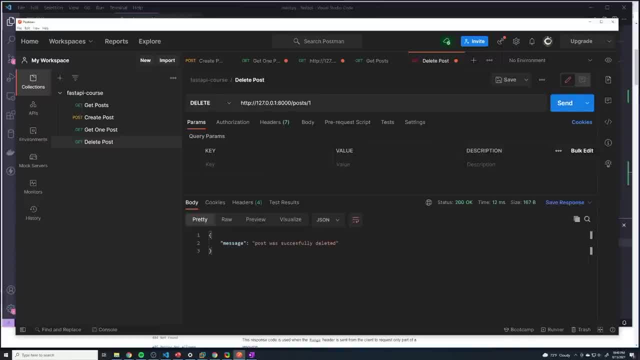 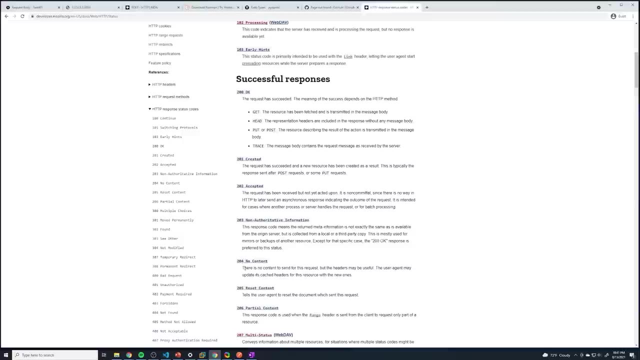 again And we see that we get the message says: post was successfully deleted. That's good. However, you'll see that the status code is 200.. And so if we actually go back to our status codes, you'll see that there's a specific status code that we should be using. 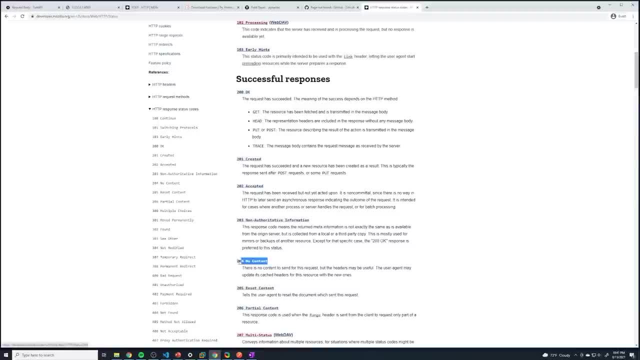 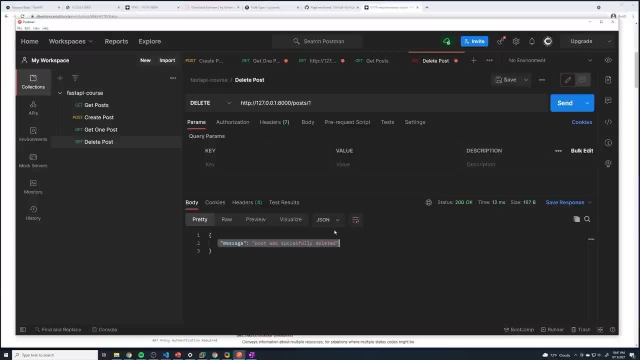 for when we delete something, And that status code is a 204.. And, like I said, you know you can read the documentation, But this is something that just you know comes with time of working with API, So you'll know that anytime you want to delete something. you. 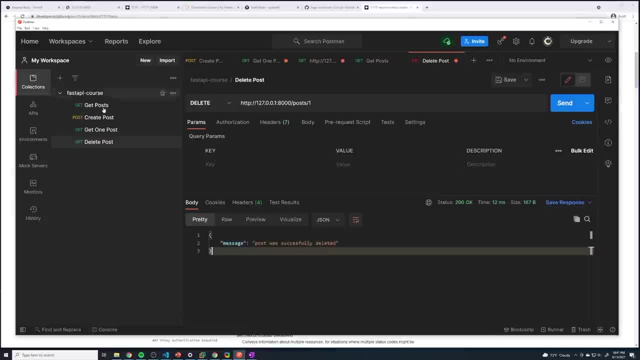 want to use a 204.. But before we actually do that, let's verify that it actually deleted it. So we'll go to get posts And I'll send a request And we can see that there's only one post. So it clearly did work. 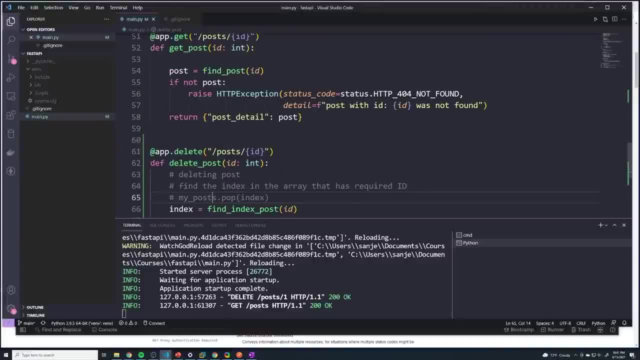 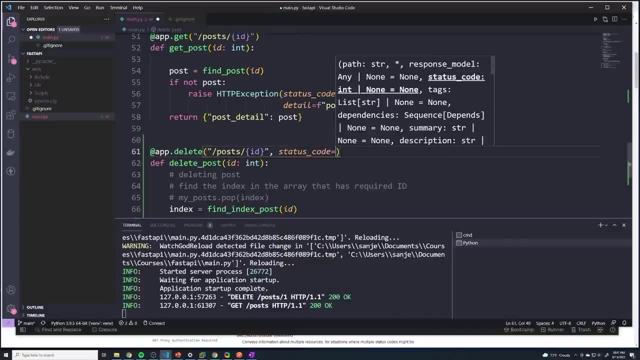 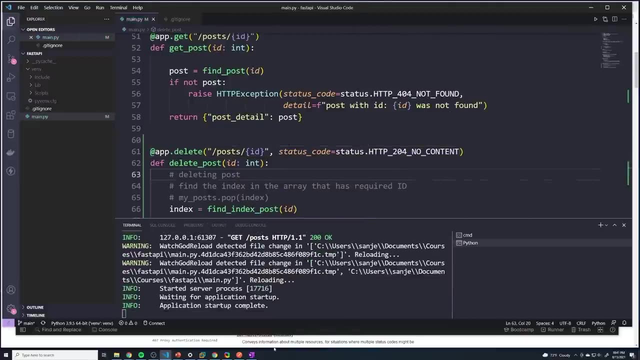 But let's update the status code. So do you guys remember how to update the status code, the default status code of a specific path operation? we just pass in status code into the decorator and then we'll do status and then we'll just get our 204.. Now let's try. 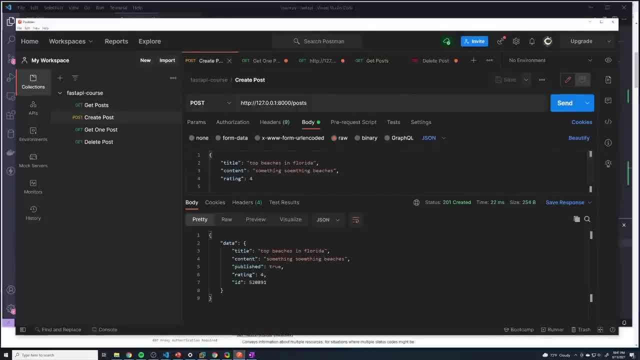 to delete something again. We'll try to delete. Where's my delete? I'll try to delete post one again. Let's see what happens. So you'll see here that we get the 204.. So everything looks good. We didn't get any data back And if we go back to our application, you'll 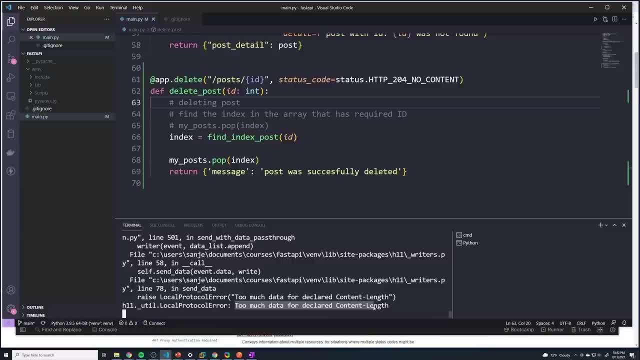 see that we got a, an error which says too much data for declared content length, And what's happening here is: I actually had to look up this error, And that's because anytime you send back a 204, the idea is that since we delete anything, we shouldn't really be. 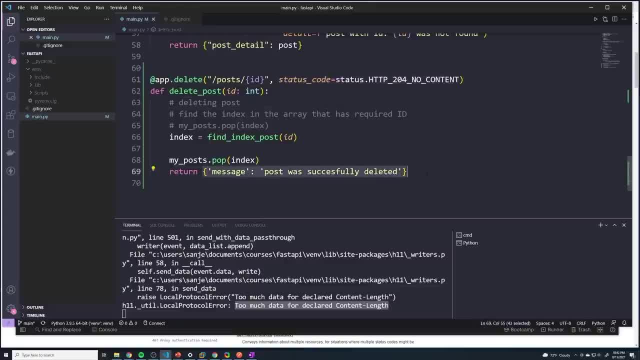 sending any data back, And so when we try to send this message back, fast API essentially throws an error saying like: Listen, you're sending a 204, we should not be sending anything back. So that's how they kind of implemented fast API. So that's how they kind of implemented fast API. 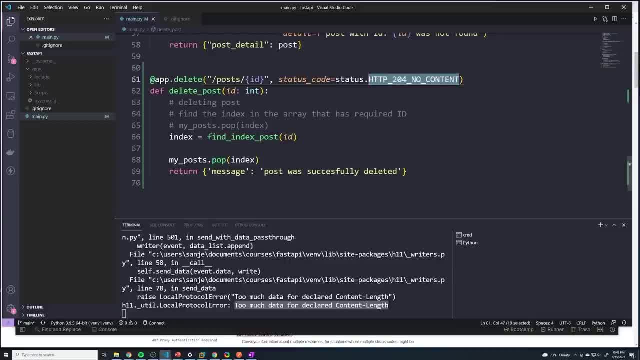 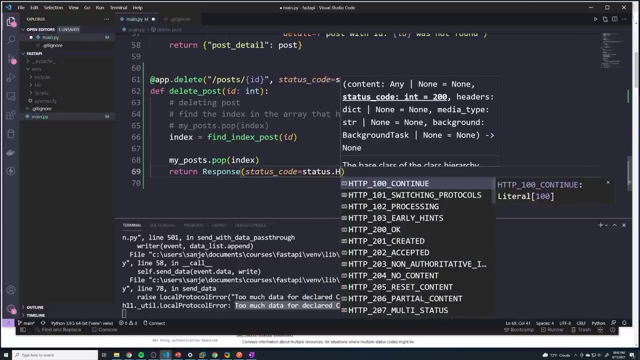 And so the what you should be doing is, if you want to do, if you, what we should do is actually just delete this. we should grab the response And then just pass in status code: status: HTTP 204.. Right, So basically, we don't want to actually send any data back. 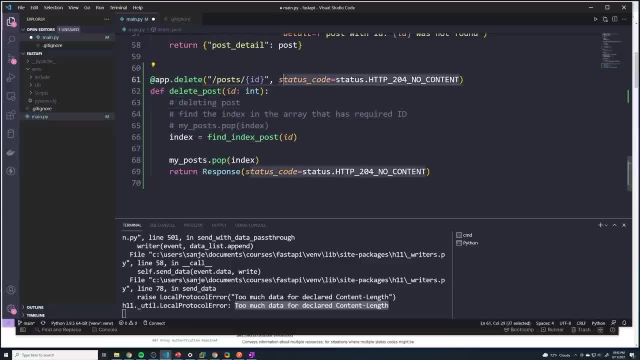 Anytime someone delete something, we just want to send a 204. And then one of the requirements for that to work is that we don't send any data back. I know it's a little confusing. If you actually just Google this error, you'll probably get. 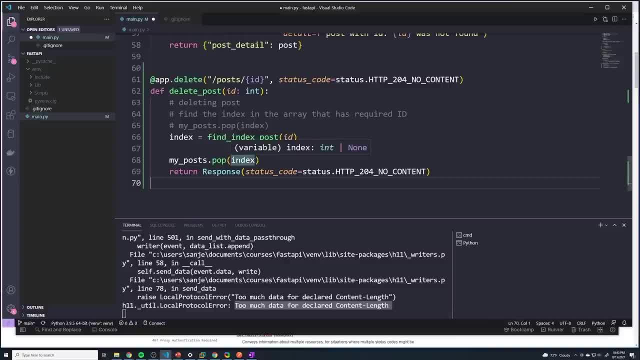 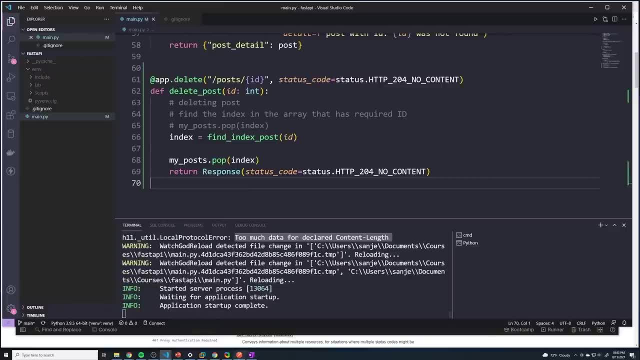 better explanation. But 204, when you delete something, you don't want to send any data back. That's kind of the expected result. So let's try this again. Let's send it. Alright. so we got the 204, no data comes back And no errors. So that's all we have to do. So 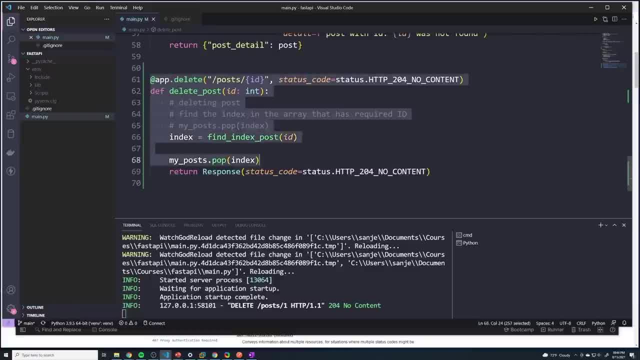 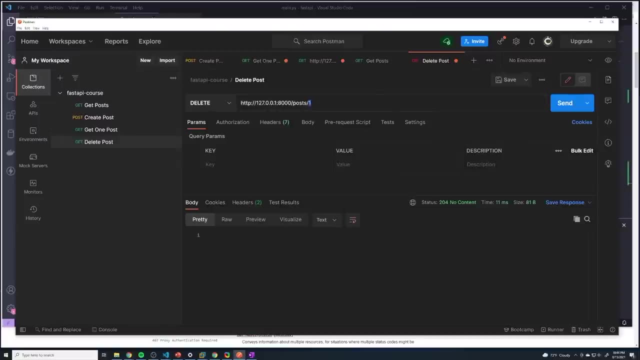 this is just something special that you have to do for delete within fast API. Just keep that in mind. It's more of just a copy, A cut and paste type scenario. However, before we wrap up this delete video, we are still running into one tiny issue. If I try to grab a an ID that doesn't exist, let's see what. 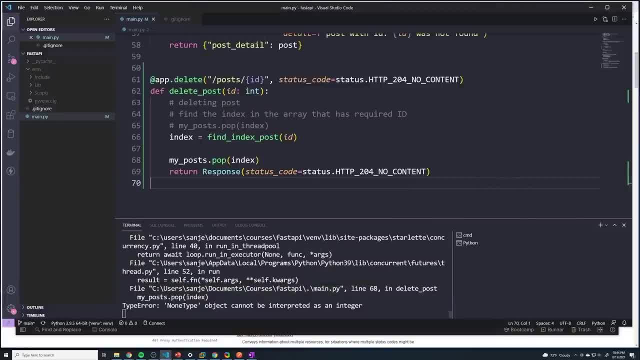 happens. Well, now we get a 500 error. And we get an error because, well, none type object cannot be interpreted as an integer. So since we tried to grab the index from this find index post, it's going to return nothing because there's no post. 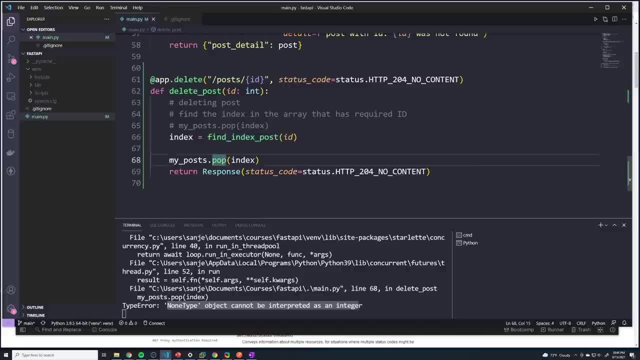 That has an idea of five. so we get nothing. And then we try to pop with an index of none. that creates an error. So we need to put in a simple if statement to actually catch that scenario. So we'll say: if index equals equals none, so return none if it doesn't exist. 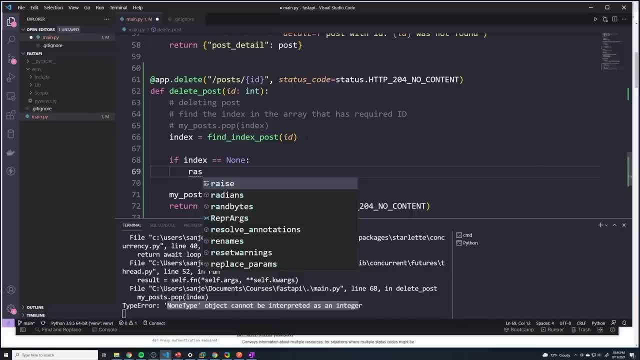 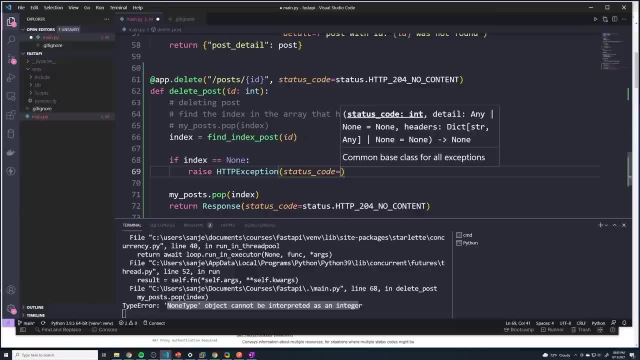 What are we going to do? Well, we're going to raise an exception again, So we can use that raise HTTP exception And we'll just say: status code equals. In this case, we want to send a 404 like we normally do. 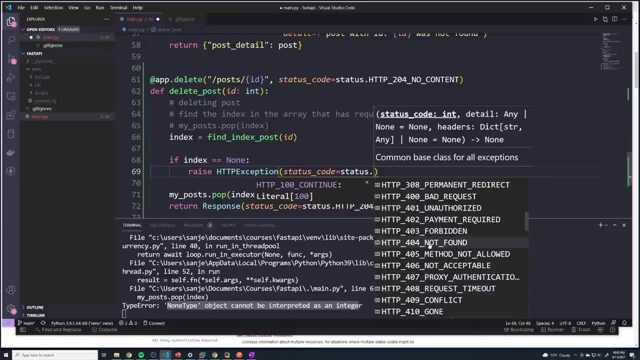 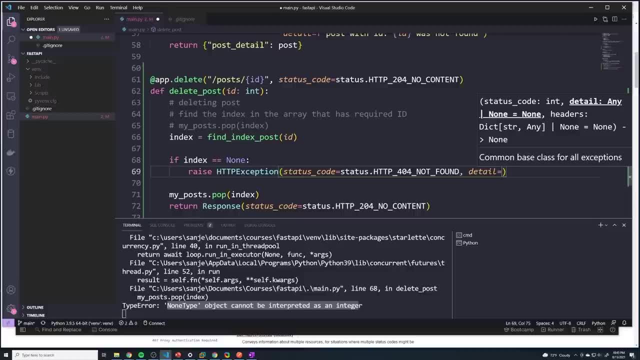 we'll say status: dot HTTP 404.. And then we can send a detailed message. So in this case, you know, we'll do once again another F string And we'll say: post with ID pass. the ID does not exist. 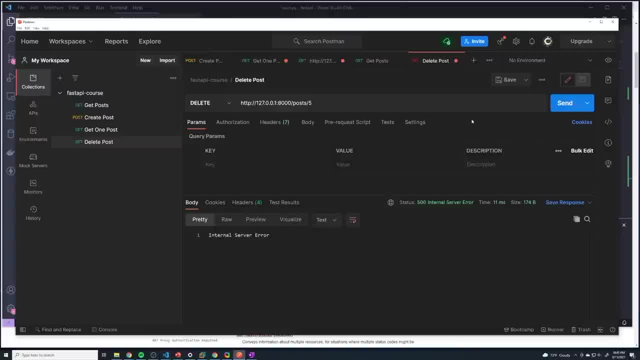 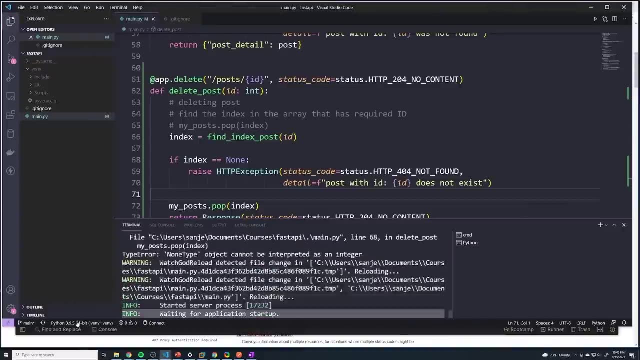 So let's try this out. Perfect 404 post with ID doesn't exist. Let's just make sure we didn't break the original functionality. We delete it. Perfect, And let's just double check. there's no errors. There we go. So everything looks good to go, guys. So we'll wrap up this video And 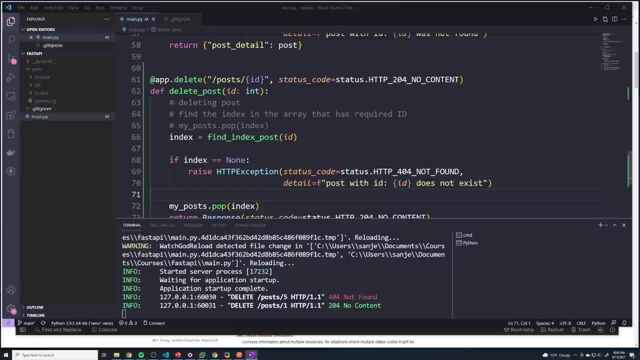 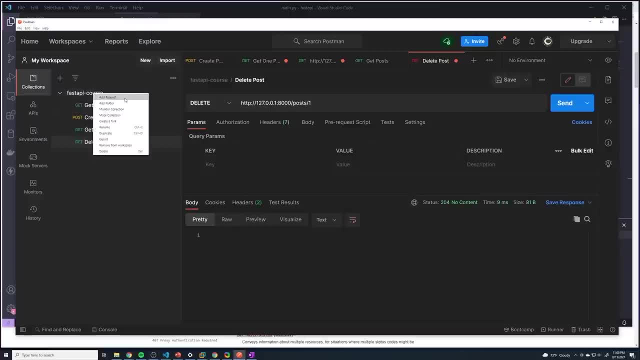 then in the next video, we'll take a look at how we can update posts. Alright, guys, we're almost done with all of our CRUD operations. The final one is update, So let's create a new request. We're going to call this update post. 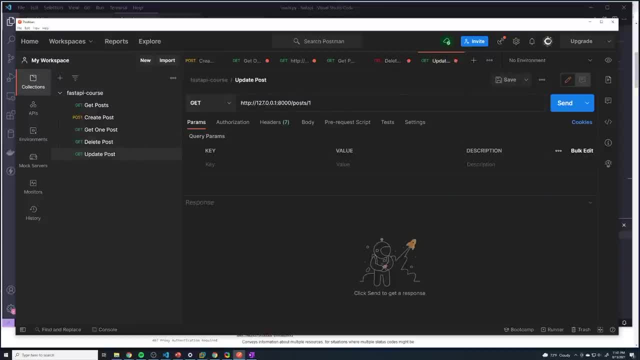 I'm just gonna grab the URL from the delete post because it's going to follow the same exact structure, So we're going to pass the ID of the post that we want to update. Now, since we are updating it, we need our front end, or in this case postman, to actually send the 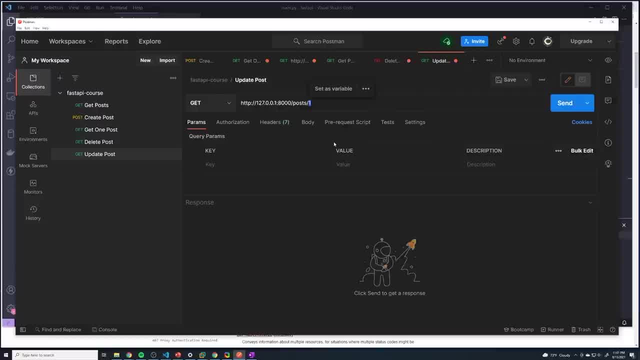 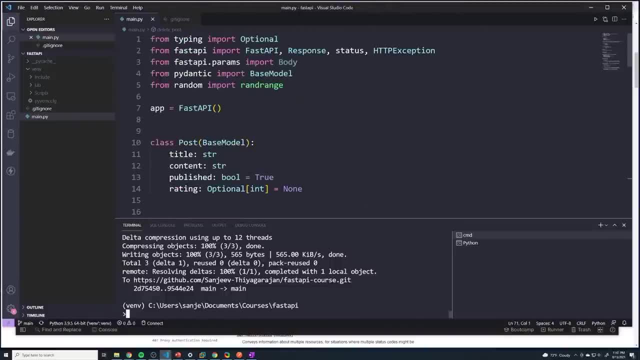 data that we want to update with. So, since we are working with posts and we take a look at our structure of our posts, it's very simple. we just have title content And then you know published as well. if you want to add that in ratings as well, And I'm actually going to remove- 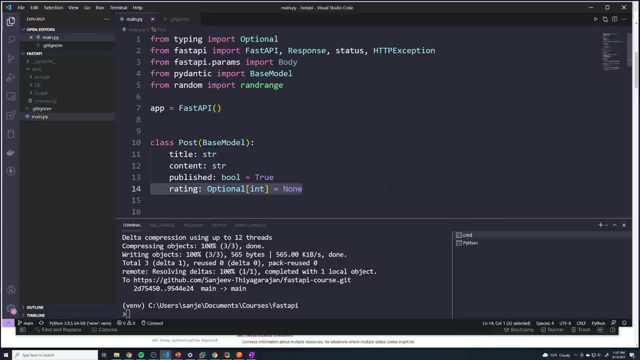 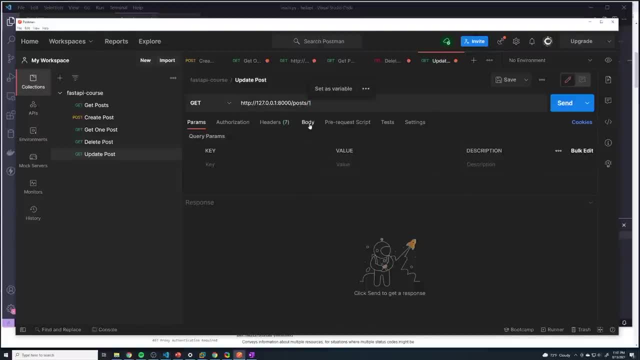 that. So I don't actually want to have that. I'll actually we'll keep it in for now, But we'll definitely remove that a little bit later on And so if I go back to postman, we can go to our body and then provide all of those fields. So we'll go to raw and then JSON. But this is just like. 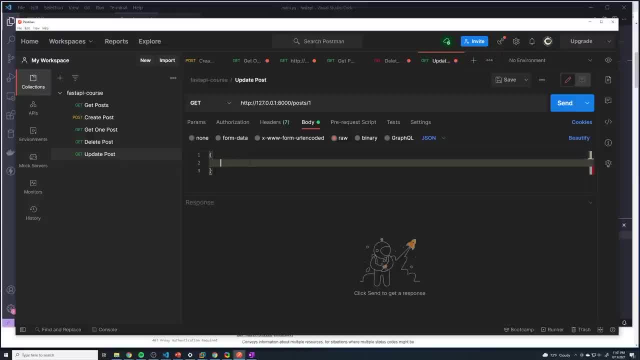 when we were trying to create a post. we just pass that data in, And so here we'll get the title And we'll give it a new title. So updated title. So this, this, this update request, is just going to update the title. Now we are going to use the put method. 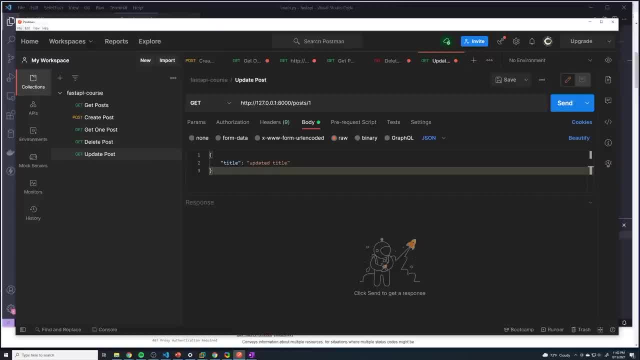 So with put method, we have to actually pass in the data for all of the fields. right, we want to pass in what the final post will look like after we update it. we don't just want to pass in the fields that we want to update. So if I go to 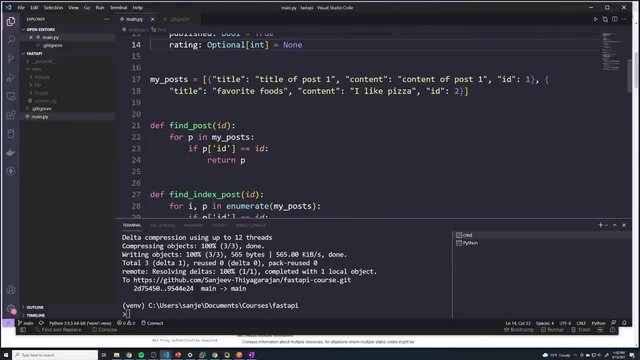 let's say, you know, post one right, we have the title and then we have the content. So if I wanted to update just the title, right, I would make sure that I pass the content as well. So I'm 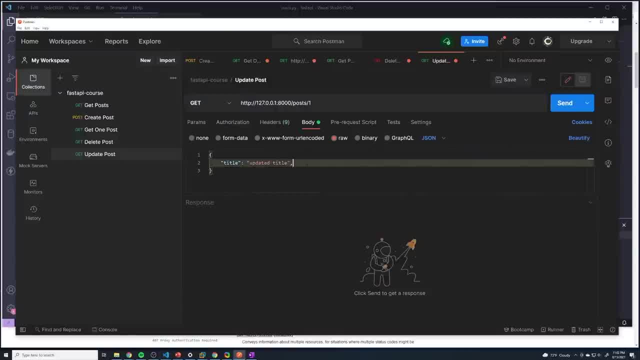 just going to copy this. Since we're not updating, I'm just going to send back the same exact content, Right, And then this is going to be a put operation, And so this is what the request is going to look like. Now let's go to our 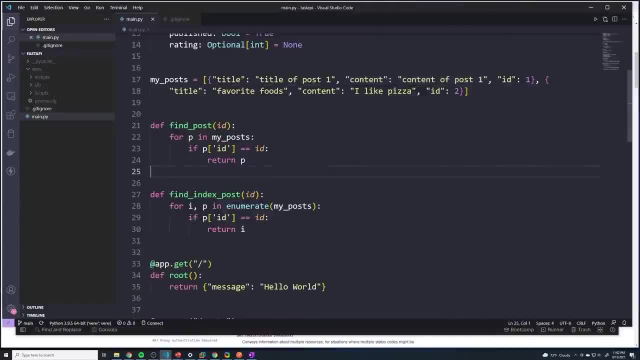 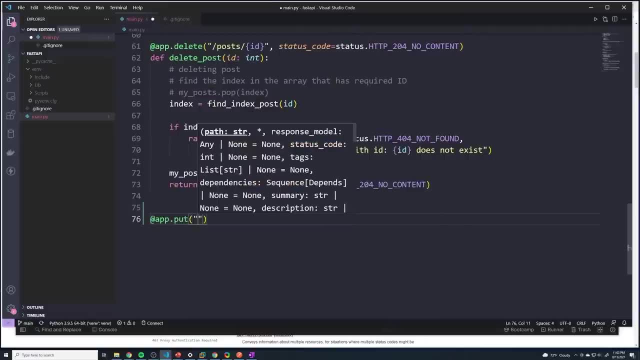 code And let's actually create our path operation for that. So here we're going to do app dot put. It's going to go to post the D And then we'll define our function. I'm going to call this update post, We're gonna get the ID and I'm going to convert that to an int And then one other. 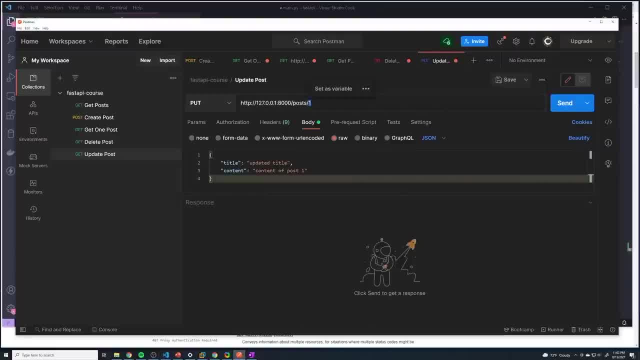 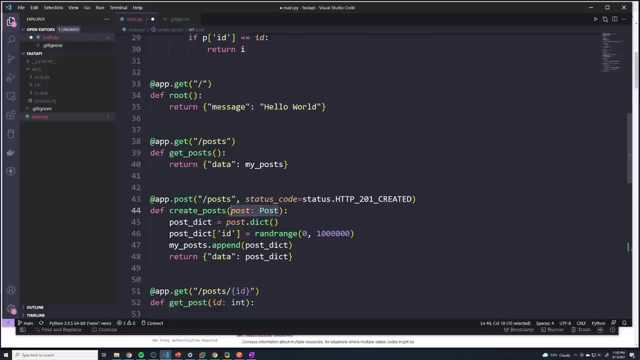 thing right, Because we are receiving an update. we're going to call this update post And then receiving data from the front end. just like we did for creating a post, we want to make sure that it adheres to a very strict structure, So we get to use. so I want to use our schema again so that 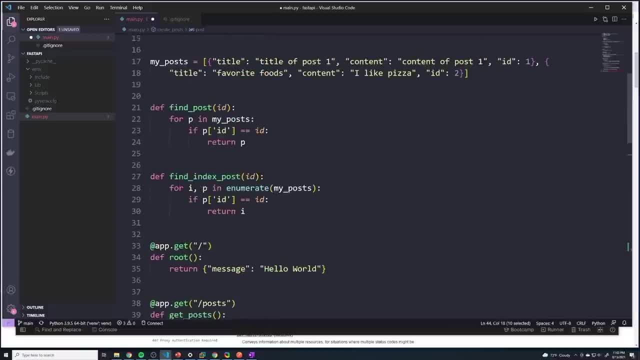 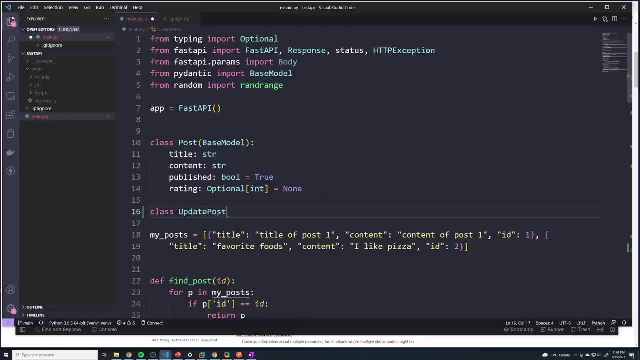 the front end can't just send whatever it wants to. Now I can create a new model called class, you know, update, post, And then we can pass in all the fields that we expect. However, it's going to be the same thing as the post, because we expect the title content and then any of the other. 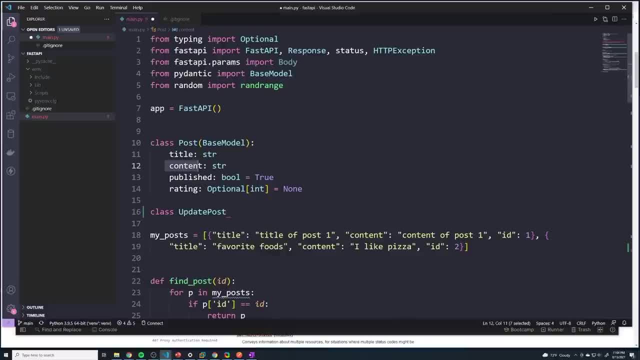 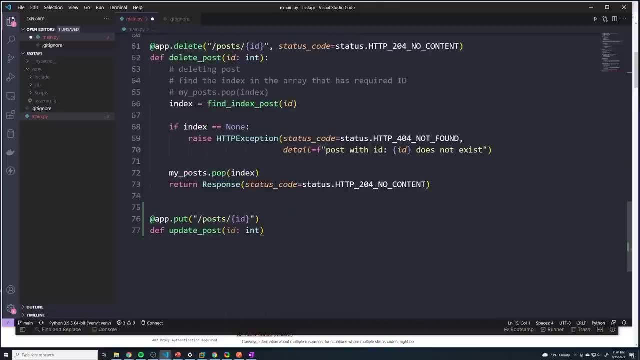 fields that we expect, And then we can pass in all the fields that we expect, And then we can pass in all the fields depending on what we want ultimately. but it's going to be a post, So it doesn't make sense to create a new schema. we can just use the pre existing schema. And so here I'm. 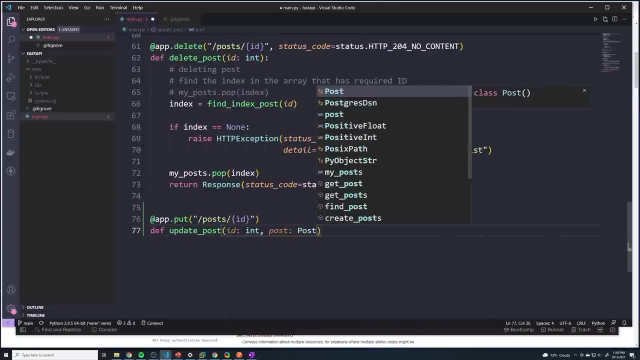 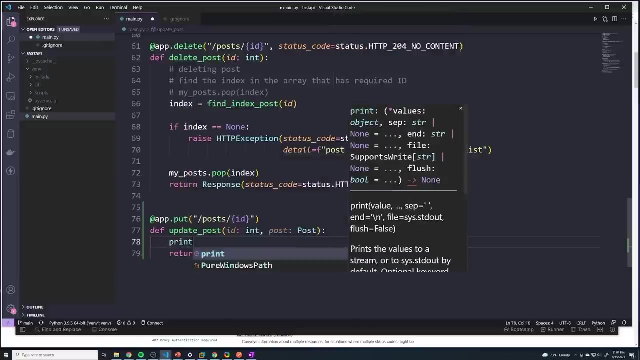 just going to pass in post and make this type of post so that it's going to make sure that the request comes in with the right schema. And then, for now, I'm just going to hard code the return to be a message And I'll just say updated post. And then here I'm going to do a print. let's just 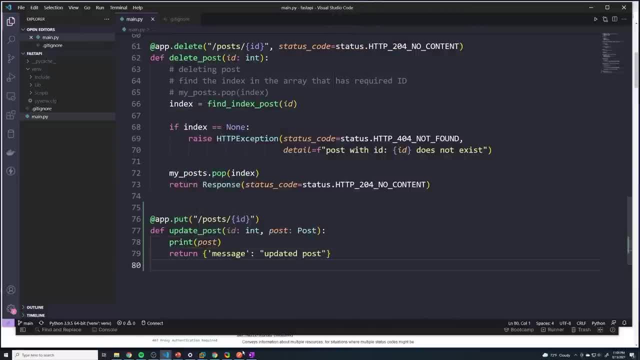 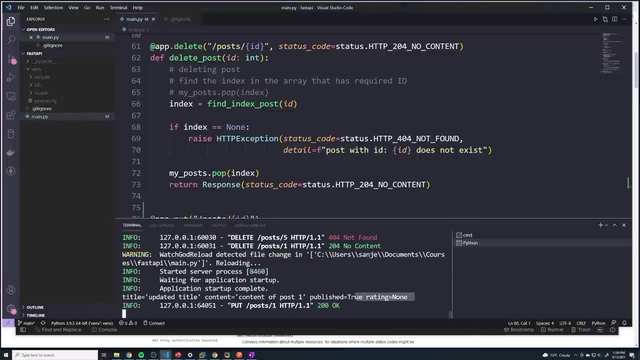 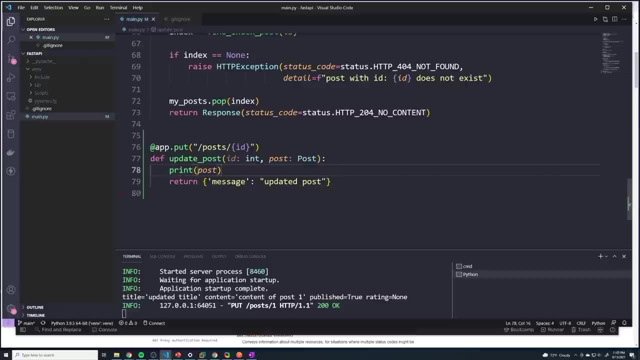 see what the post looks like. Alright, so we were able to extract all of that data. So perfect. And then what we're going to do now is there's a couple things. So, first things first, I need to find the index, that of the data, And then I need to find the index of the data, And then I need to. 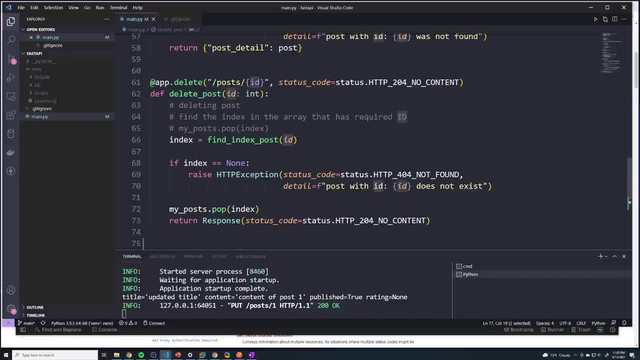 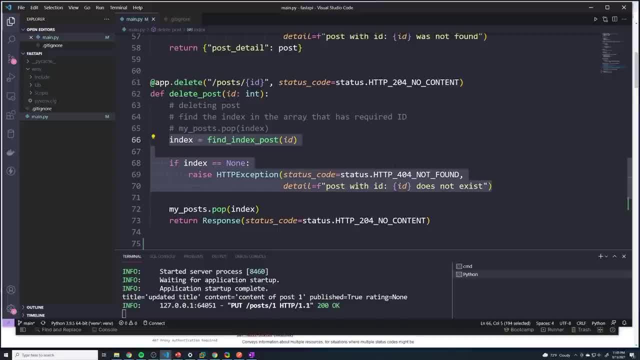 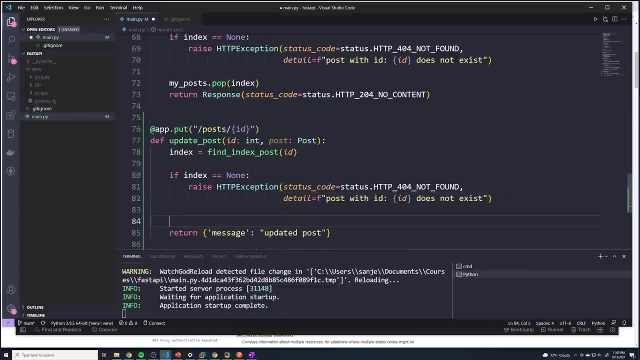 right here, Because if that ID doesn't exist, we want to send a 404.. So we can reuse all of that logic. But if we did find an index, that means we do need to update it. So what I'm going to do is: 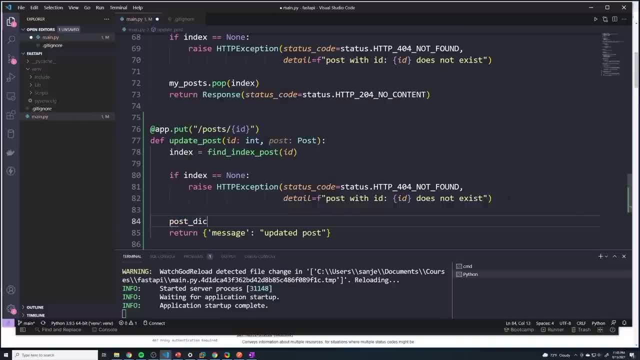 we're going to grab post underscore dict, which equals post deck. that's going to take the data we received from our front end, which is stored in post, And it's going to convert it to a dictionary. That's all it's doing. And then what I want to do. 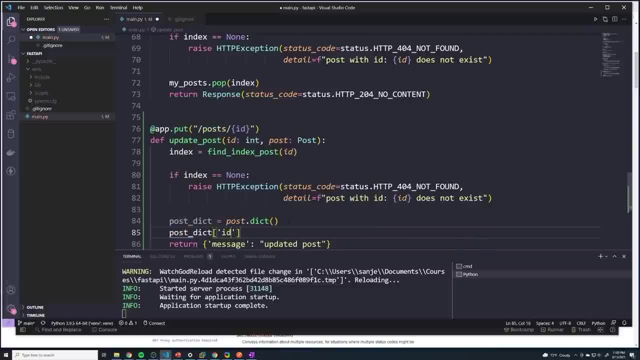 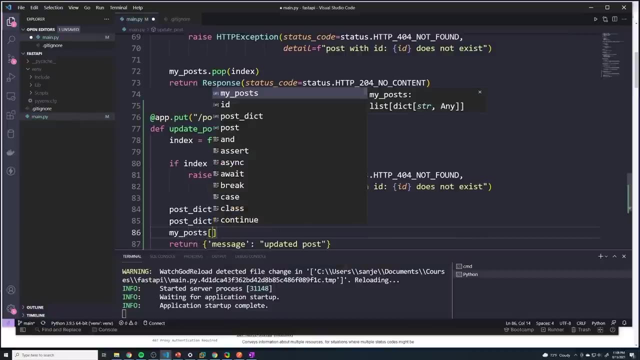 is: I want to set post underscore dick of ID to be equal to 80. So we're going to set the ID inside this new dictionary to be that ID And then we're going to say my underscore post And we're going to pass in the index of the specific post we want to update and set that equal to post And then we're. 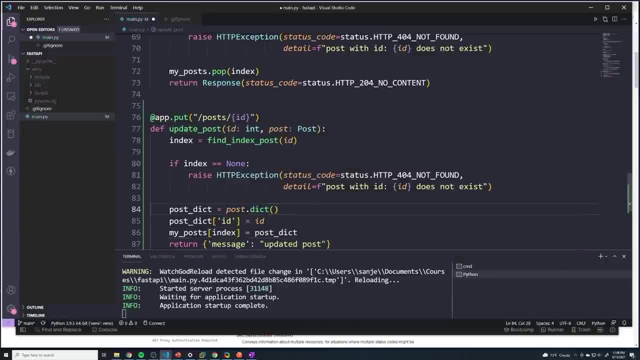 going to pass in the index of the specific post. we want to update and set that equal to post. And then we're going to pass in the index of the specific post. we want to update and set that equal to post. underscore deck. And then, lastly, we're going to return, I'll say data And we're going to return. 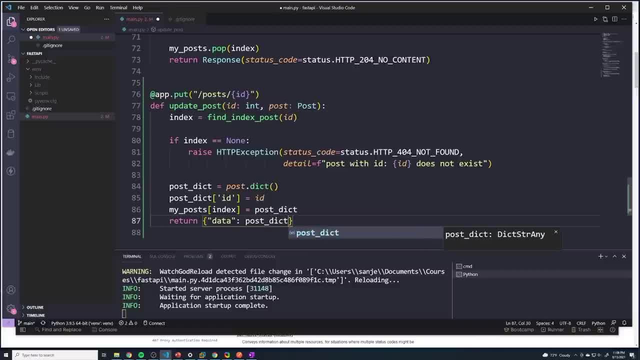 our new post, which is going to be post underscore deck. So let's just quickly recap what's happening. So, first of all, the user is going to send a put request to the specific ID of the post he wants to update And we're going to just do a quick check. So we're going to see if we can find. 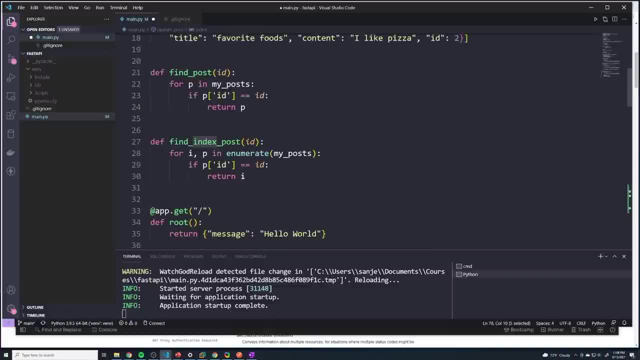 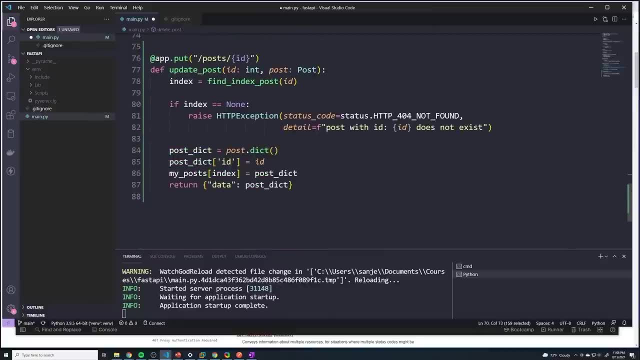 what is the index of that specific post within my my posts, Ray? if it doesn't exist, then we're just gonna throw a four or four. if it does exist, whoops. if it doesn't exist, we're gonna throw a four or four. If it does exist, well, first thing we're gonna take. 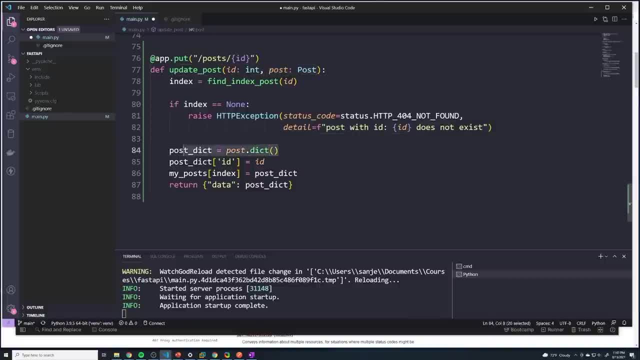 all the data we received from the front end, which is stored in post. we're going to convert it to a regular Python dictionary And then we're going to add the ID, so that this final dictionary has the ID built in, And then we're going to say: for the post within index, we're going to just replace it. 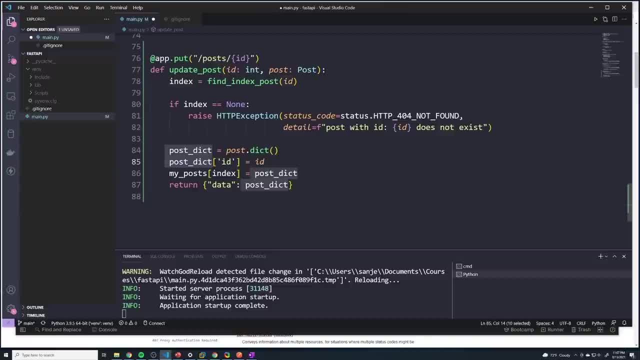 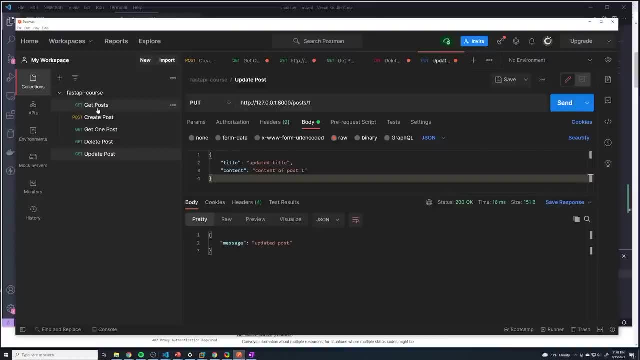 with our new post underscore dict. So that's how we update that specific spot In the array, And so let's give this a shot. So, if I do get all posts right, we can see we have post one and then the title is title of post one, And then let's go to our update And we can see that. 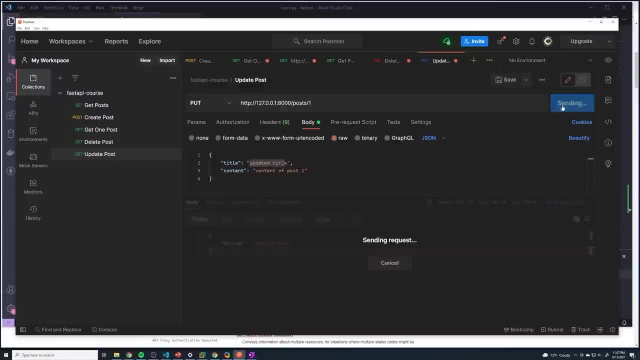 we're going to change the title to be updated title And let's see if that works. Okay, so it looks like it worked. We got back the new post, So let's do a get all posts again And let's see if. 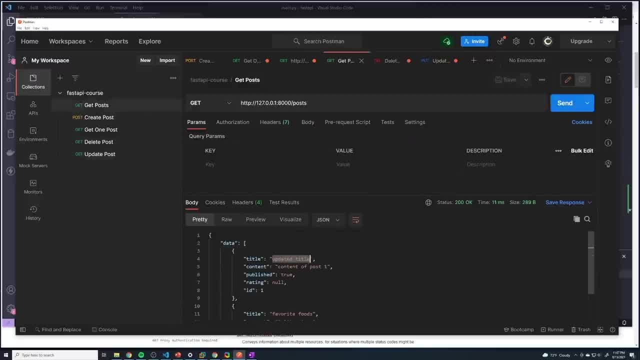 it actually did update And we can see that it did in fact update. Now, just to just to make sure everything else is good, Let's also change the the content. So let's say this is the new content, Let's send an update, And then we're going to run this again And we 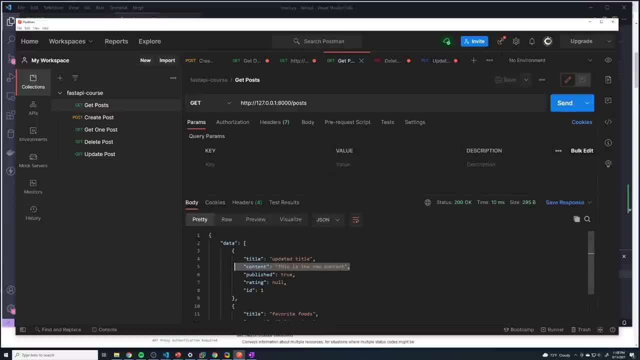 could see that the content is updated. So now we're able to successfully update each and every post And that's going to wrap up all of our CRUD operations. So you can see that building out an API, building out your CRUD functionality, is fairly straightforward within fast API. 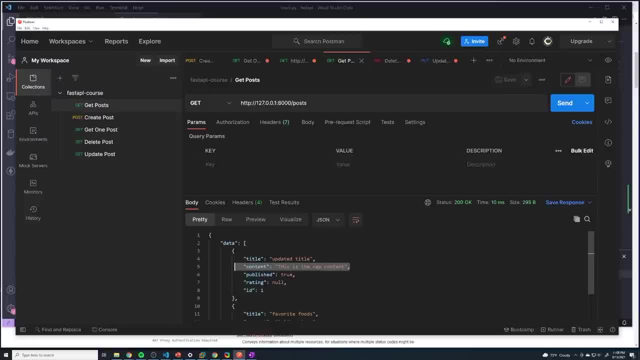 We've got one more lesson where we're just going to restructure our code a little bit, just to make things a little bit cleaner, And then we're going to start getting to the fun stuff, which is working with databases. So I'm going to show you guys how we can actually get a Postgres database installed. 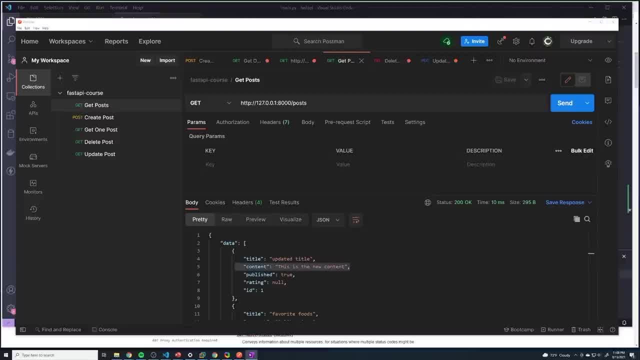 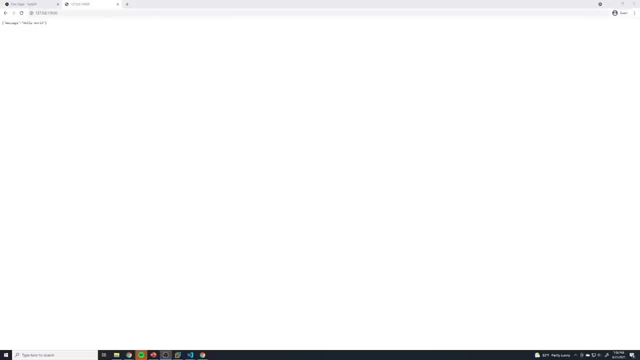 on our machines and running and then we'll actually start saving data into an actual database. In this lesson we're going to talk about one of my favorite features of fast API, And that is the built in support for documentation. So normally when you build an API, you're going to want to. 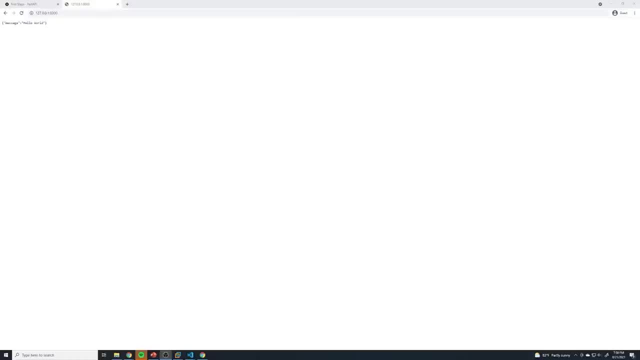 create documentation so that users know how to use it, And one of the challenges with that is that it's not exactly a simple process, And anytime you make changes to your API, you have to make sure that you update your documentation, And it's very easy to forget to do that With fast API. fast API. 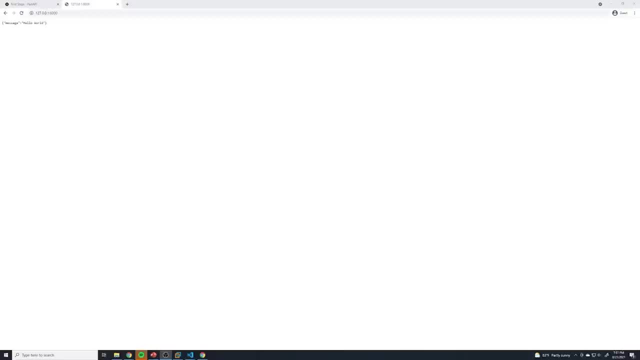 automatically generates the documentation based off of the path operations that you've defined. So it does it all for you And you don't have to write a single piece of code to actually get the documentation in place. And so to actually see the documentation, you just go to the normal URL. but 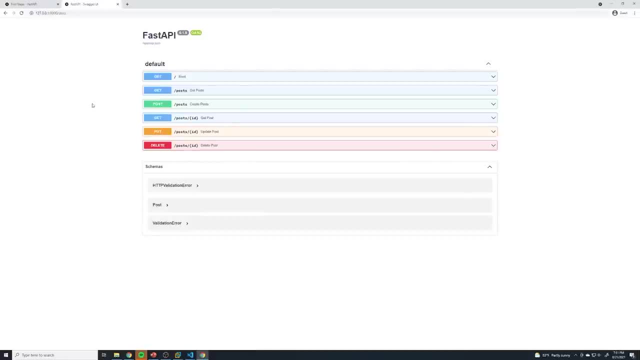 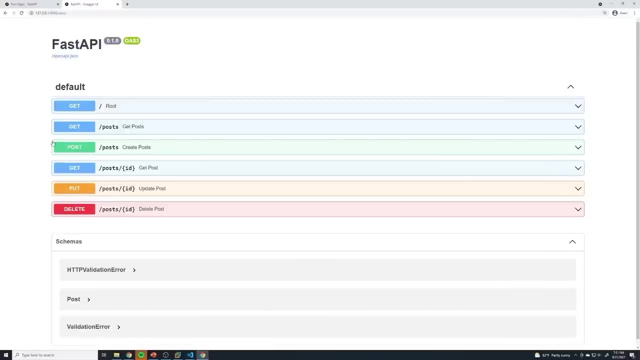 you just do slash doc, And so this is going to show you the built in documentation powered by swagger UI. And so what's really nice is- and if you've ever looked at the documentation for some other API's, you may have noticed something that looks similar to this, And that usually means that they used swagger UI as. 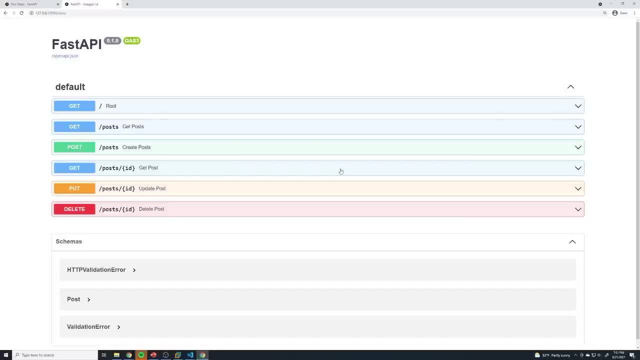 well, So fast. API has built in swagger UI support and it automatically generates all of the routes and the documentation for all of your paths. And if you take a look at all of our operations, our path operations, we've got the one for getting all posts. we've got the one for creating posts. we've 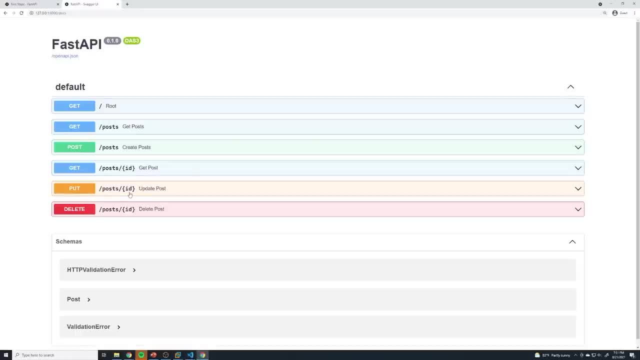 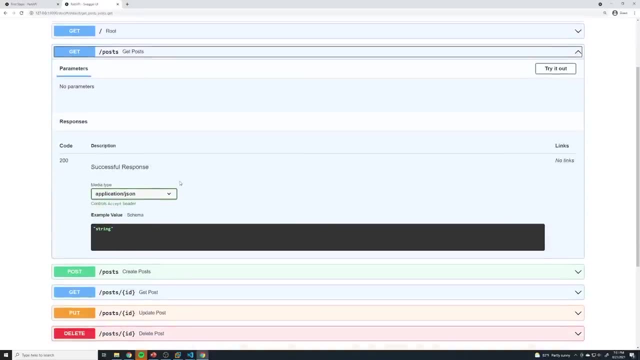 got the one for getting an individual post. we've got the one for updating an individual post as well as deleting a post, And what's really cool about this is, if we do the hit the drop down right, it's going to show you how to use this specific path or how to use this specific API endpoint. So if you want to, 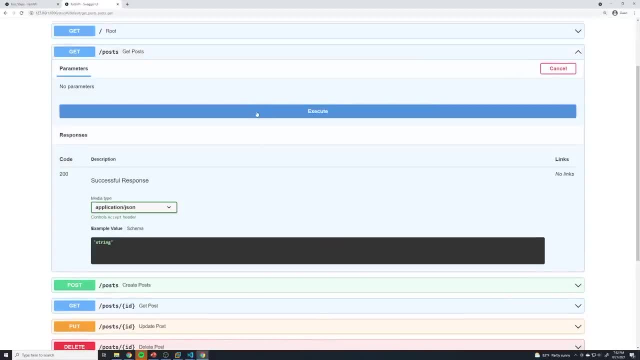 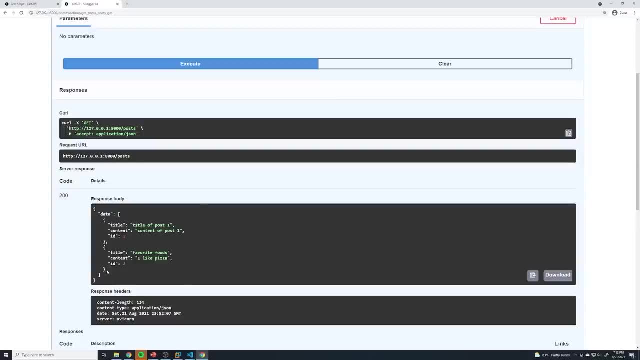 actually try it out. you can do that, So you could say: try it out, And then you can just hit execute Right, And so now it actually ran the query against our API server And it shows us what the output is. So these are the two documents that we have, or the two posts that we've created. 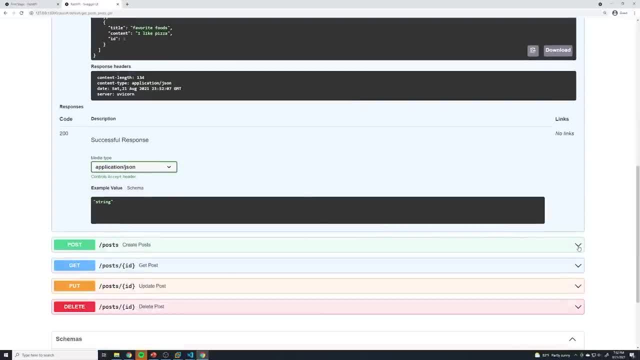 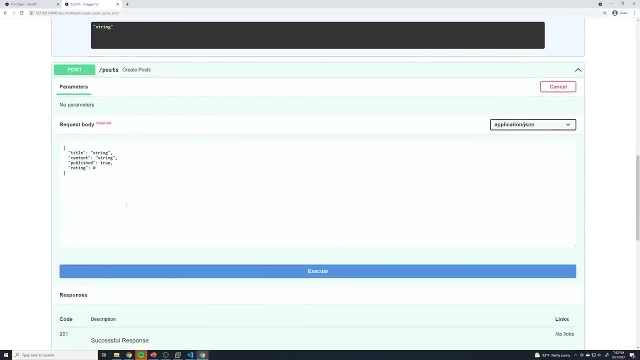 We can do this with all of the API endpoints. So if we want to create a new post, it's going to give you an example of the data that we can pass in, so we can try, try it out, And then it's going to give us all the fields that we have to pass in, And then we can just 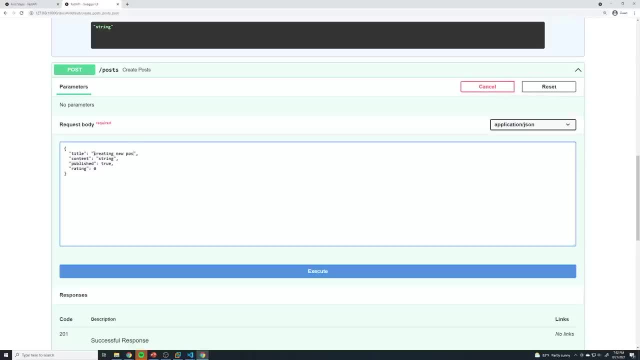 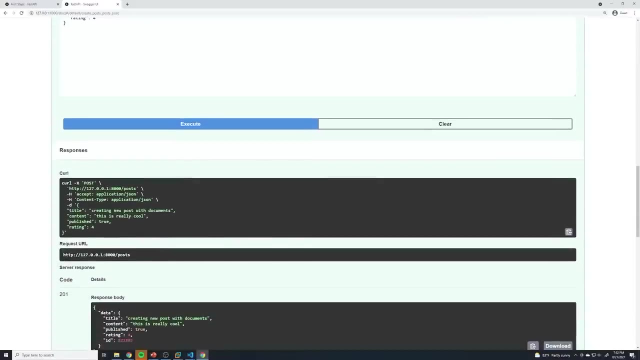 customize this. So if I want to say creating new post with documents, And then I'll just for content, I'll say this is really cool. We'll give it a random rating. we hit execute- Right, it actually runs. that it's going to show. 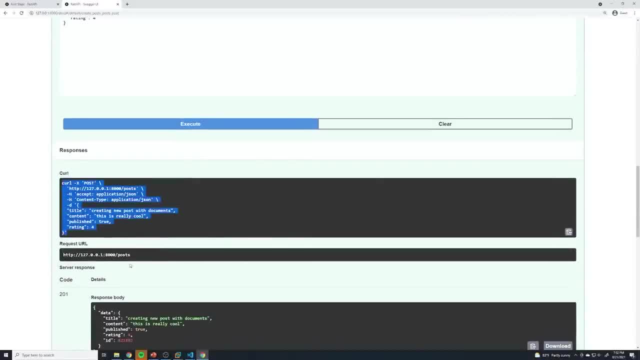 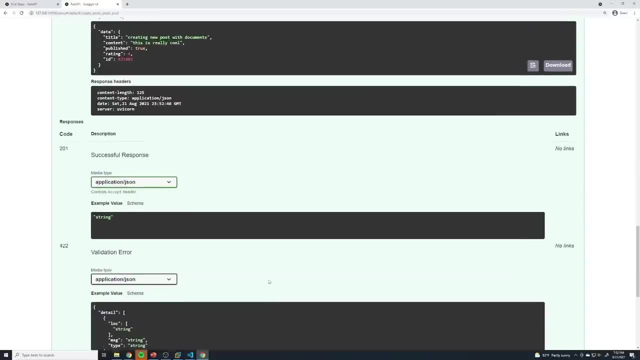 you how to perform the same actions using curl as well, And then it's going to show you the data that we got back from our API server And we can see that we got a 201 response code, And so I want you guys to just kind of play around with this, get familiar with it. So there's going. 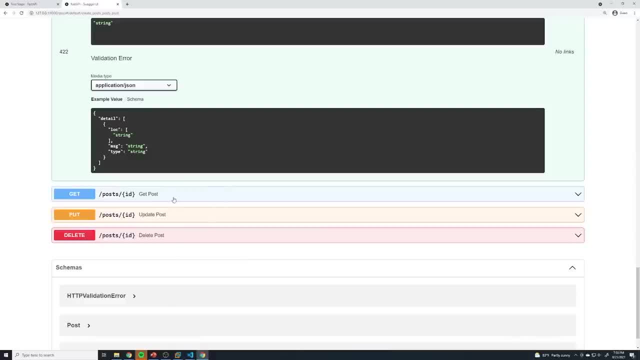 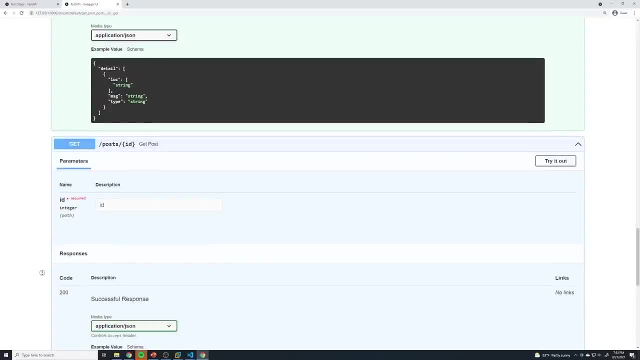 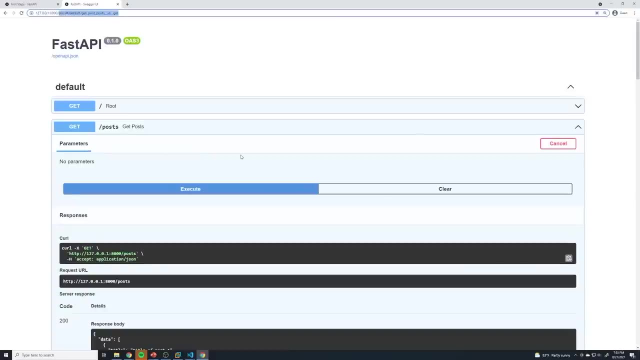 to be times where you may not even have to use a tool like postman. you could just test things out using swagger UI in the built in documentation. And what's even nicer about this is that we have built in support for two different types of documentation. So this is using swagger UI. 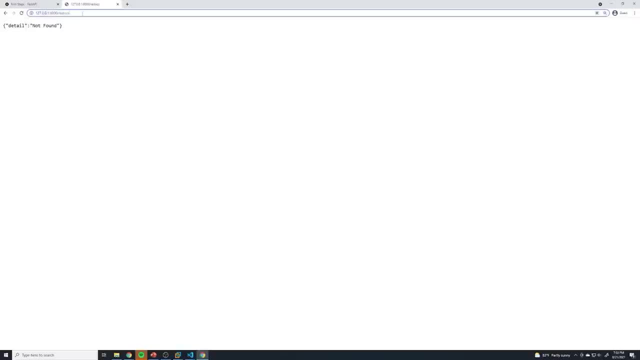 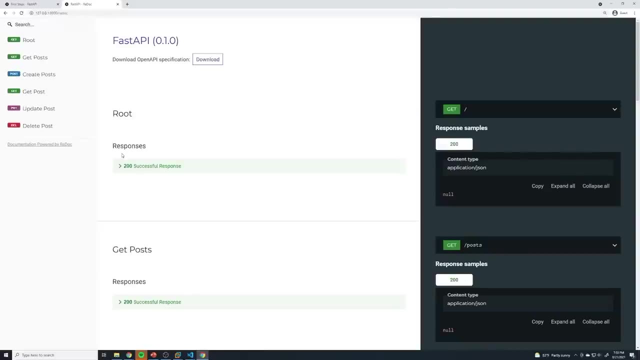 But if you use redox- I'm sorry there shouldn't be an S at the end- it's just redock. Right, you could see a different format of the documentation using a tool called redock, So it's going to fundamentally do the same thing. It's just a different documentation tool, So it's. 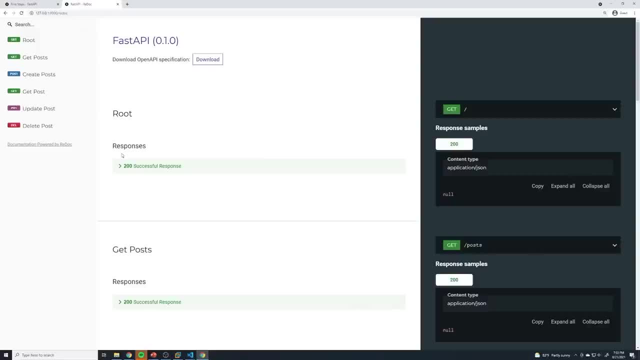 going to look a little different. Feel free to use whichever one you ultimately prefer, But by having it automatically get generated by fast API, you don't ever have to worry about updating anything. So if you take a look at like create post: right, we've defined the pieces of data. 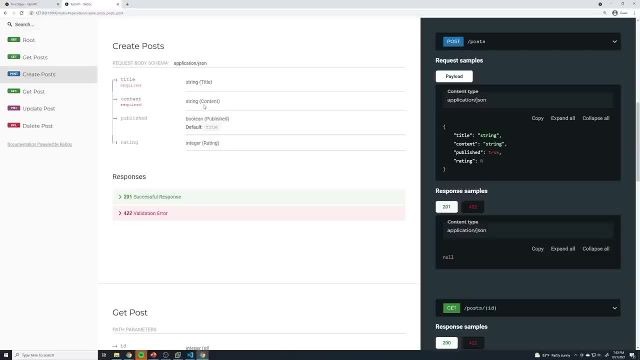 that we need And in the future, if we decide that the user needs to pass in another field- maybe like the date that they wanted to get published- it'll automatically update this. you don't have to tell it. you don't have to manually go in and update it yourself. 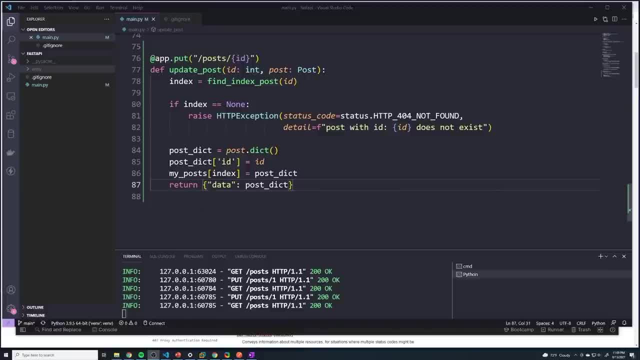 All right, guys. so we're going to make one slight change to how we structure our code, And what I want to do is, instead of just having my main file with within my base project directory, I want to actually create a folder called app, So that's going to store all of our application. 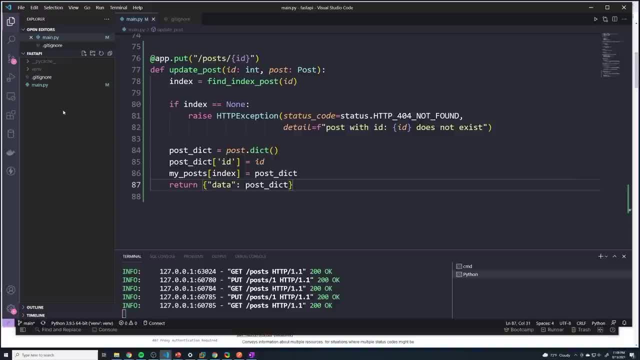 specific code and then put that main file in there. So it's a very small change, But we do have to change a couple of things to make sure that it doesn't actually break anything. So I'm going to create a new folder And I'm going to call this app, And so this in Python, if you. 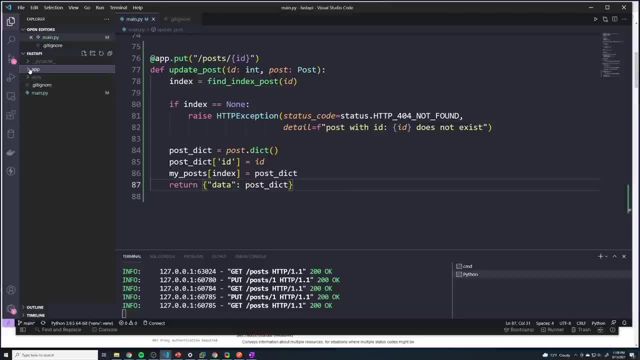 aren't too familiar with how Python works. Python has a concept of packages, And a package is nothing more than a fancy name for a folder. However, for something to properly act as a package, Python requires you to create a dummy file, And this: 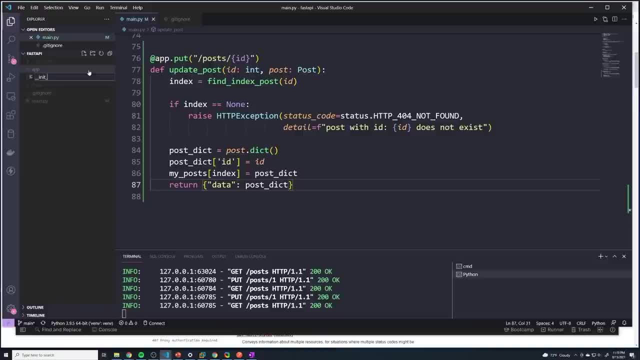 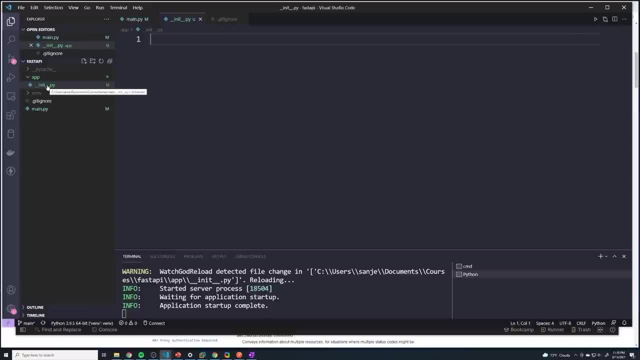 file is called underscore- underscore init. underscore- underscorepy Right, And so that's going to turn this into a proper Python package. Just know that you have to add this file. you don't have to put anything in the file. But anytime you create a new folder, just make sure you create. 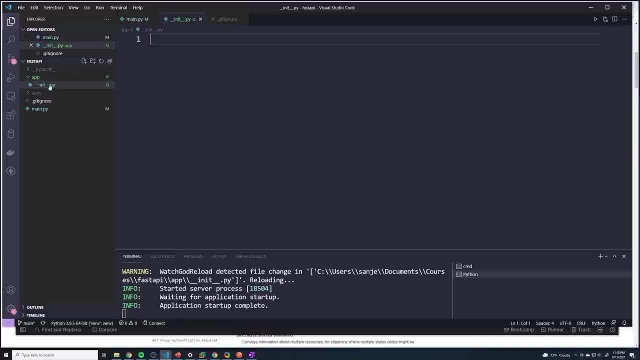 a new one And that's going to ensure that it is in fact a Python package. So now that this is an actual Python package, we can just drag this main file into our app folder, Right, and then now we're going to get an error And that's perfectly okay. So we're going to cancel out of this And I want. 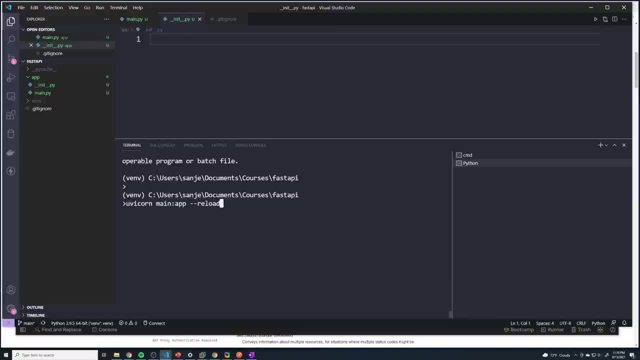 you to take a look at the command that we run to start our application. So the command to start our application was: we do UV corn, we do the name of the main file, which is just main, And then within main. if you take a look at what's the name of our fast API instance, it's called 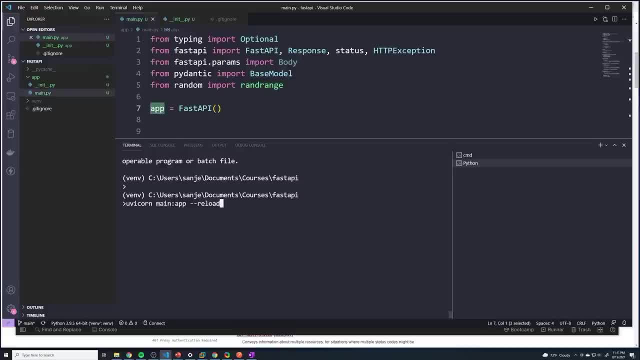 app. However, now when we run this command line, this command, it's going to look for a file named domain. However, there's no file named domain within our base project directory because it's now been moved into app. So to actually reference the main file that's inside of a Python package. 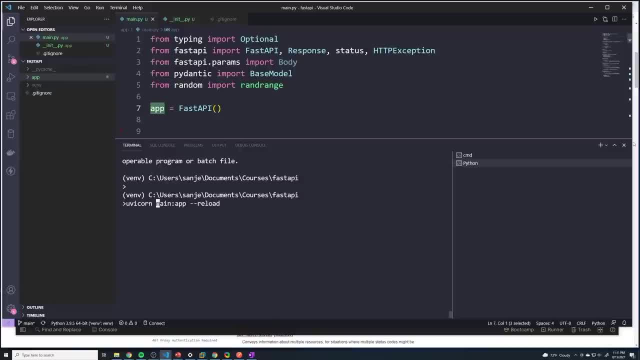 it's pretty simple. You just put the name of the package beforehand. you do app and then dot. So it's going to tell UV corn to look inside the main file And then you're going to see that it's inside the app directory for a file named main. So then we go in there, we see the main file And 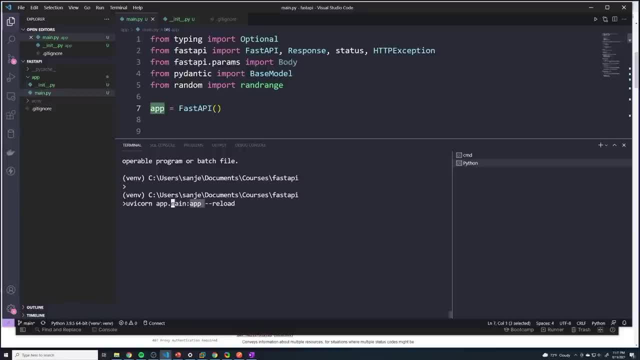 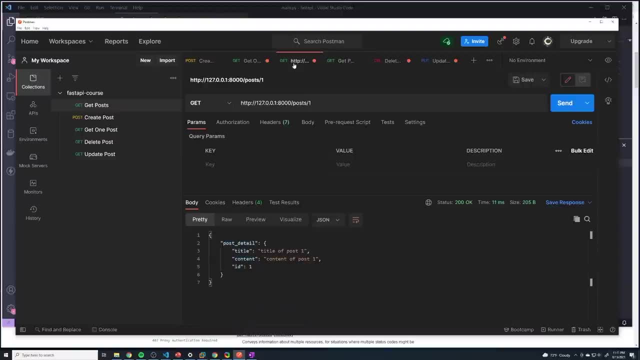 then, within our main file, we look for the app instance, which is our fast API instance right here. Let's give this a shot. Let's see if we broke anything. It looks like everything started up fine. I'm just going to do a couple of requests, So this is going to be just get an individual post. 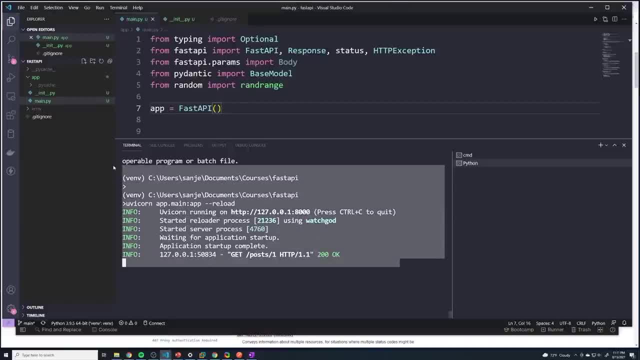 Looks like everything is good. I just want to make sure that there's no errors. And yep, everything looks good. So I think this is just a little bit better of a way to structure our application. we're going to put all of our app code moving forward inside of this app. 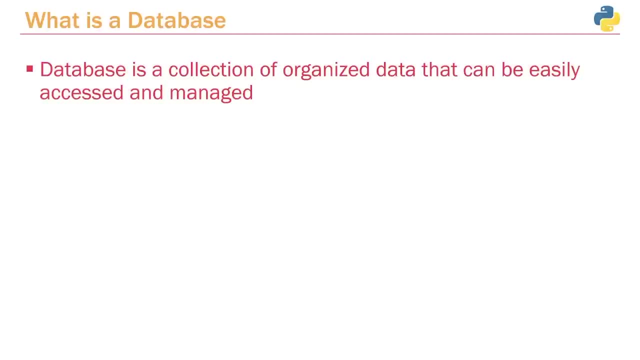 directory so that we can keep everything else separate. I think at this point we have a basic understanding of how to work with fast API and how to set up basic routes and work with path operations. Until now, we've been storing all of our posts in memory And I think we've made it to 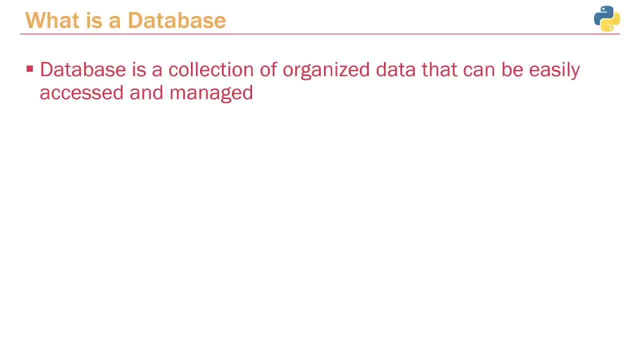 a point where we are ready to now start working with databases. And so, if you don't know what a database is, a database is a collection of organized data that can be easily accessed and managed, And so, when it comes to any kind of application related data, so things like users. 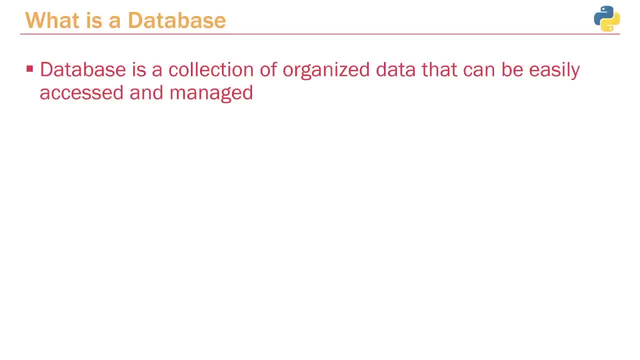 that have registered posts that have been created. all of these pieces of information are going to be stored within a database, So it's going to be stored on disk so that we can retrieve this information at a later point in time. Now, when it comes to databases, we never actually interact. 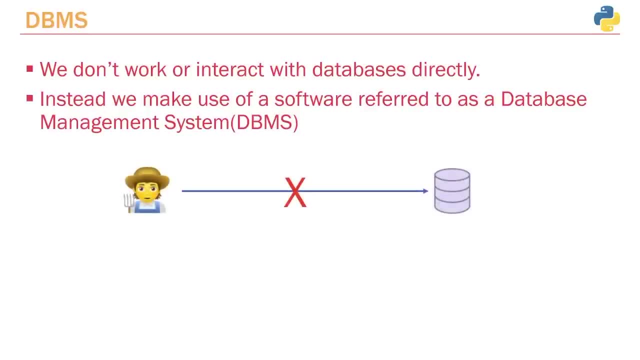 with the databases directly. Instead, what we have is a database management system that's going to sit in the middle. So when we want to perform an operation on a database, we're going to send that request to a database management system. that management system is then going to. 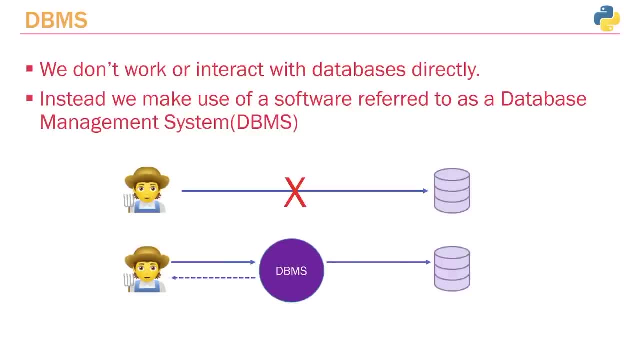 actually perform that operation and then it's going to send the result back to us. So we never talk to the databases directly. Instead, we have a piece of software that sits in the middle and acts as the brains behind the database. Now there's two major branches of databases. 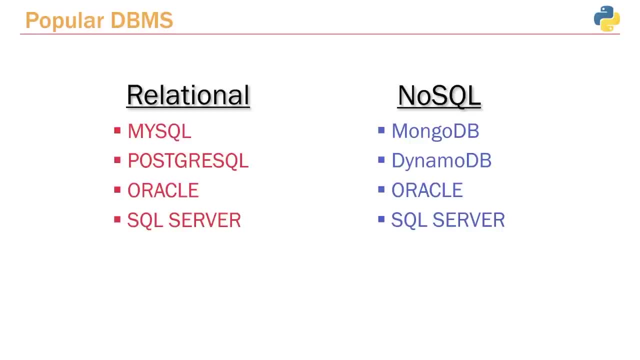 there's relational and NoSQL databases. relational databases are usually SQL based databases And we're going to cover that in the next slide or so, But these are just some of the more popular relational and NoSQL databases that you guys have probably heard of. 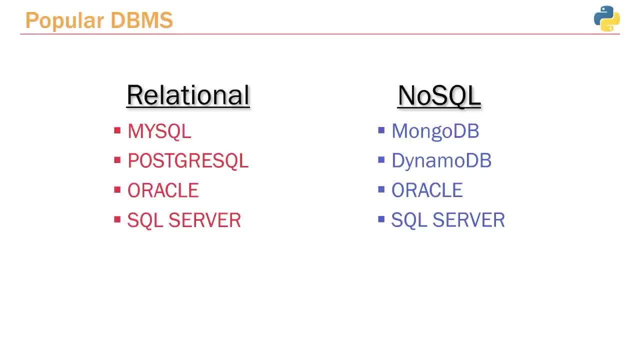 In this course, we're going to work exclusively with relational databases And, more specifically, we're going to work with Postgres. Now, if you ultimately want to learn how to work with MySQL or Oracle or SQL Server or any of the other databases, keep in mind that at the core, they 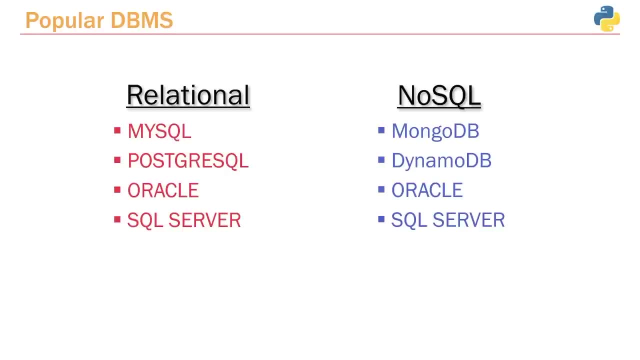 are fundamentally no different than Postgres. you know, 90, I would say 97% of the things that we cover when it comes to Postgres is going to be almost identical in all of these other databases, because they all, at the end of the day, use SQL. However, SQL, there is a little bit of slight. 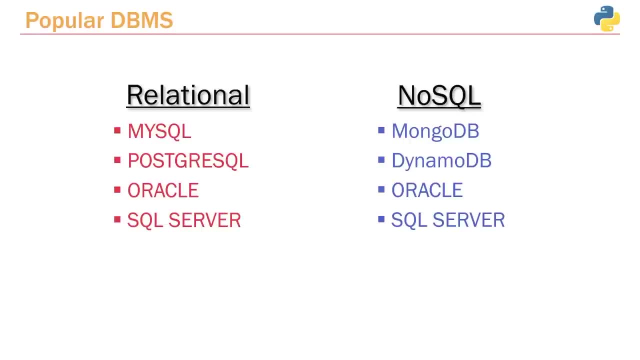 difference between the two databases. So you'll see that in each database each of them will implement it in a slightly different way. So you'll see that certain SQL commands aren't available and others, but for the most part all of the core things that we cover from a SQL. 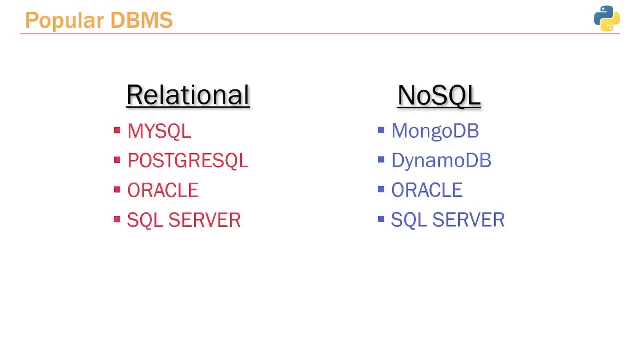 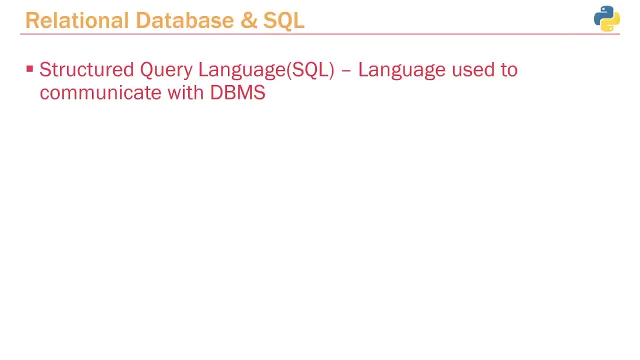 perspective is going to be applicable to any of the other relational based databases, And so let's talk about SQL now. So SQL, or structured query language, is a language that's used to communicate with the database management system, And so you know when we want to perform an operation. we're. 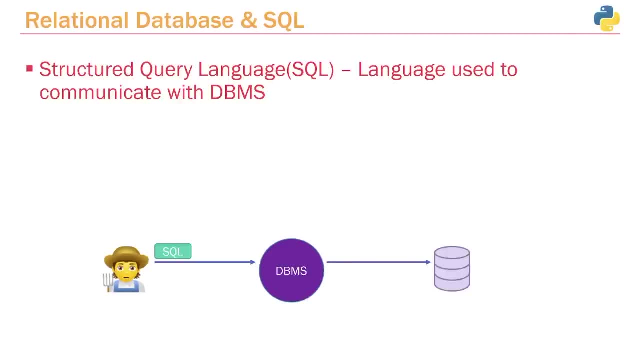 going to send a database management system. it's going to then take that statement and then perform the operation on the database, And then it's going to send that result back to us. So SQL is the language that we use to communicate with the database management system. Now, in the next video, what we're going. 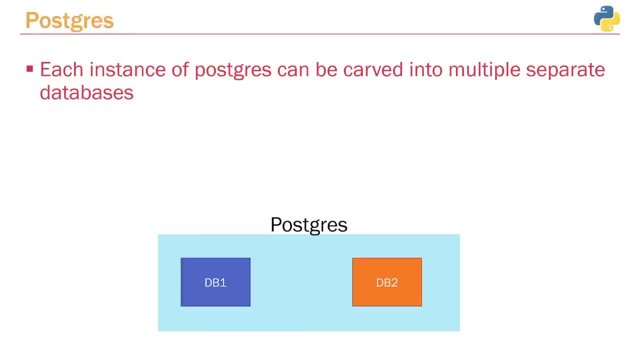 to do is we're going to install Postgres on both Windows and Mac, depending on what you're using, And there's an important thing to note when it comes to installing Postgres or really any database: When you install an instance of Postgres, what we can actually do is we can carve. 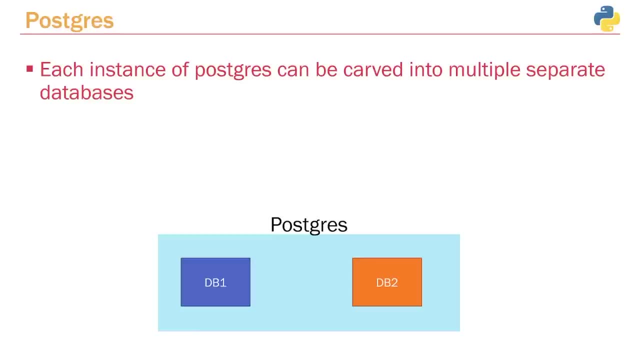 out multiple separate databases. Right, And this is kind of confusing at first, because you're thinking: well, we installed Postgres, we have a database, Yes, but what we can do is we can actually create two different databases that are completely isolated, isolated and have nothing to do with one. 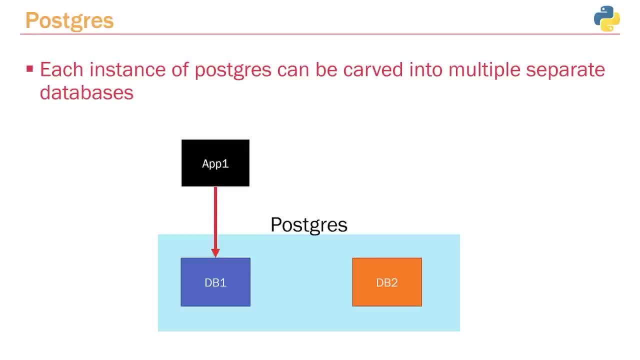 another. And that way, if I have application one, we can create a database just for app one, And then, if I have a second application that I create, this application can have a separate database as well, And there these two databases are going to be completely separate and completely isolated, so that 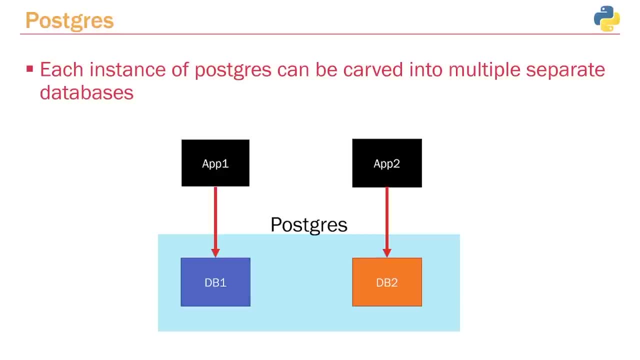 they don't step up on each other's toes. So it's pretty cool And it's a pretty awesome feature to be able to kind of carve out your Postgres instance to multiple databases And keep in mind that you don't necessarily always create a separate. 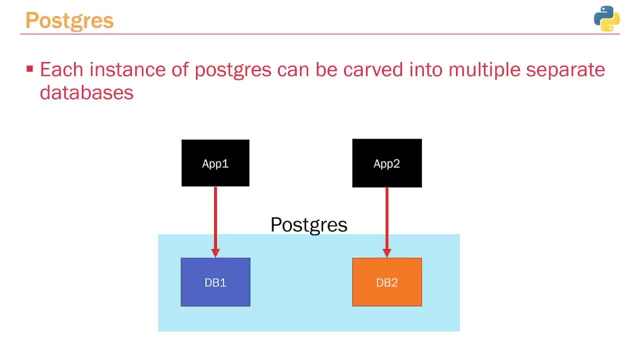 database in database instance for each application. Right, There are scenarios where you might actually create an app that's going to make use of more than one database instance within Postgres. However, those are very specific situations, maybe if you want some sort of multi tendency or things like that. However, we're just 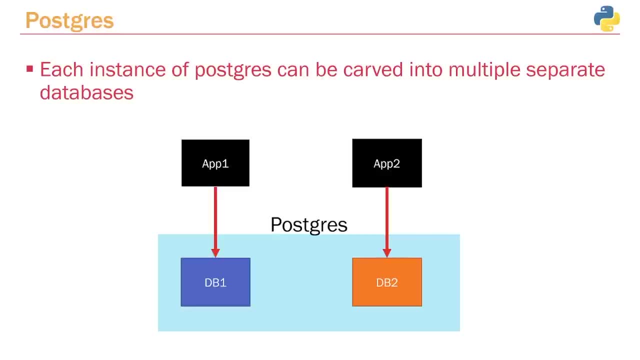 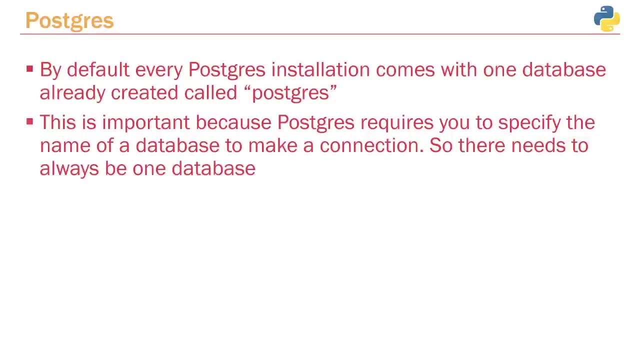 going to create one individual database instance for our application. that's going to handle everything that we need. Now, when we install Postgres, what's going to happen is that the installation process is going to create a database within the Postgres instance called Postgres. little confusing, right? It's Postgres within Postgres, But it's actually going to create this. 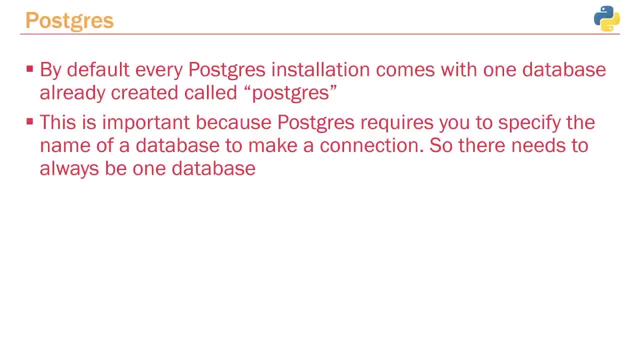 database named Postgres, And the reason we need to do this is that if you ever want to connect to a Postgres instance, what you have to do is you have to specify a database that you want to connect to, some some kind of default database that you want. 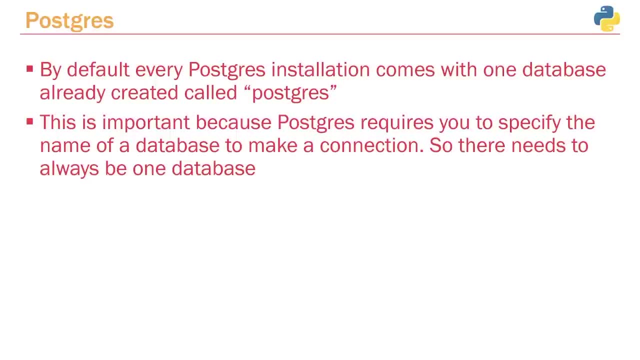 to connect to. You can't just connect to Postgres. you have to specify a database, And so that's why the installation process creates one database for you, so that you can have something to connect to. However, we won't necessarily need that instance once we create our own. However, I usually just keep it in by default, because it's not going to hurt anyone. 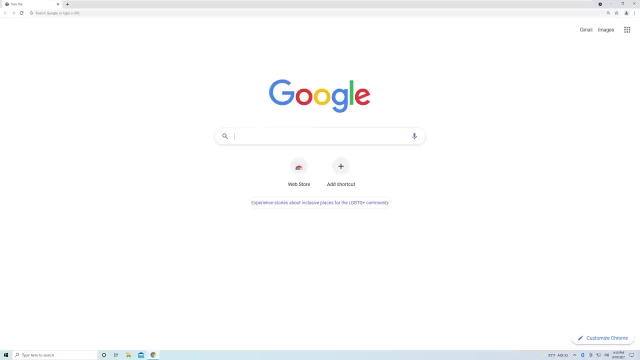 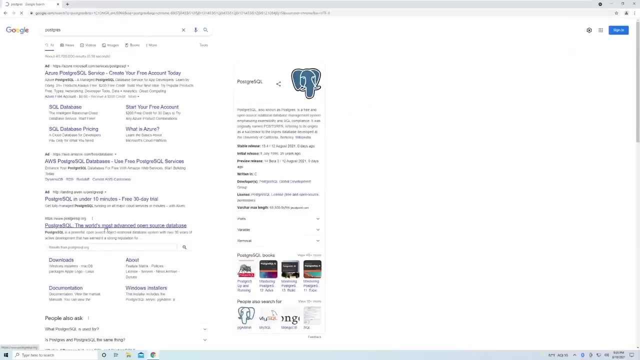 In this video, we'll take a look at how we can install Postgres on a Windows machine. So let's go ahead and just search for Postgres, And it's almost always going to be the first time we're going to use Postgres. 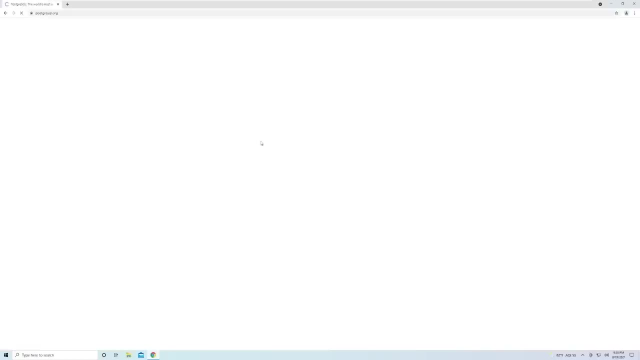 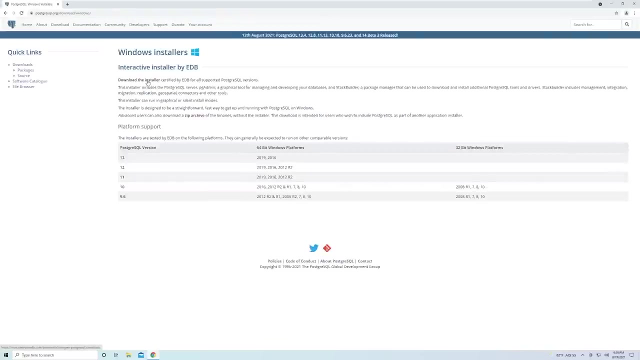 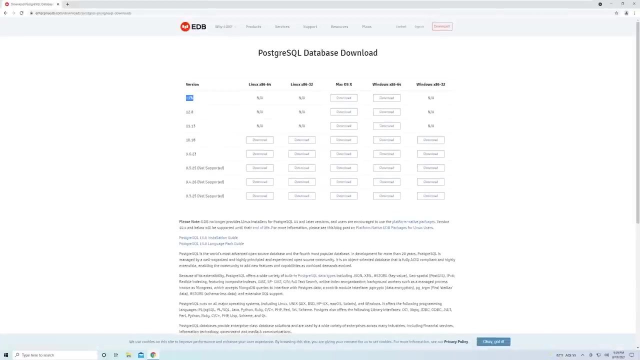 It's going to be the first instance. So just go to postgresqlorg And then we can just select the downloads button Here. go ahead and select Windows And then up here just select the download, the installer link, And so here you'll see all of the downloads options. So right now the latest version is 13.4.. So I'm going to just download that one. you may see a newer version. feel free to download that. nothing's going to really change between each version. 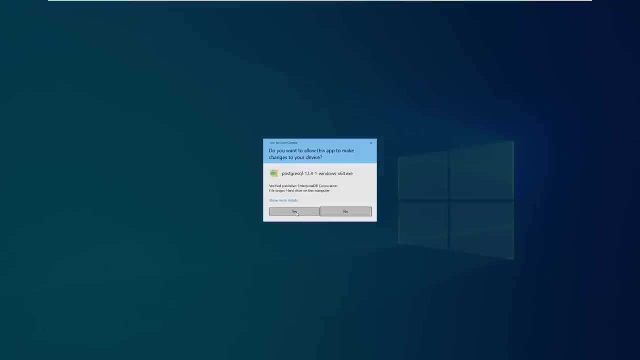 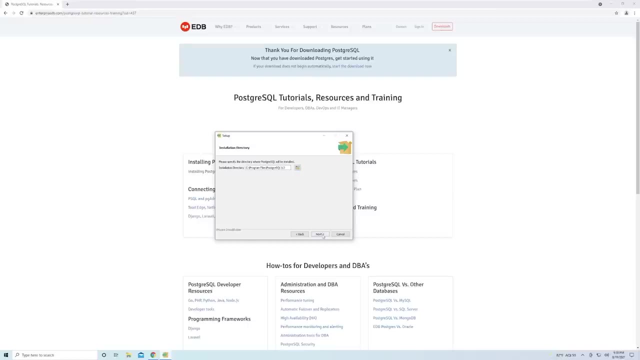 Once that's downloaded, start the installer. Once you see this pop up, just select Yes. With the installer open, select Next. you can leave the default installation directory. no one usually messes with that. Now, here you can select the different components that you want to install with your Postgres instance. So for the first thing that you have is the Postgres SQL Server. that's obviously what you want to download. 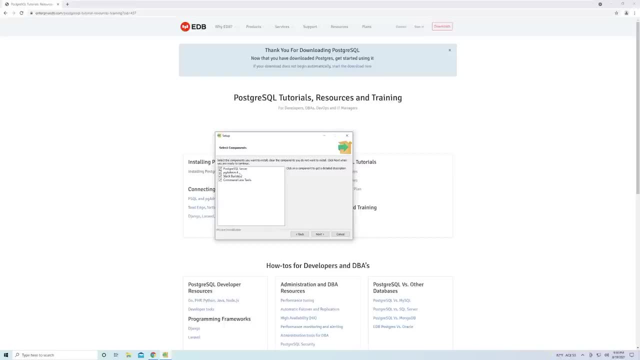 The next one is PG admin. So this is a GUI that can be used to manage your Postgres instance. we're going to be using that to actually manage Postgres, So you want to make sure that you've got that downloaded. Stack builder, this is a. 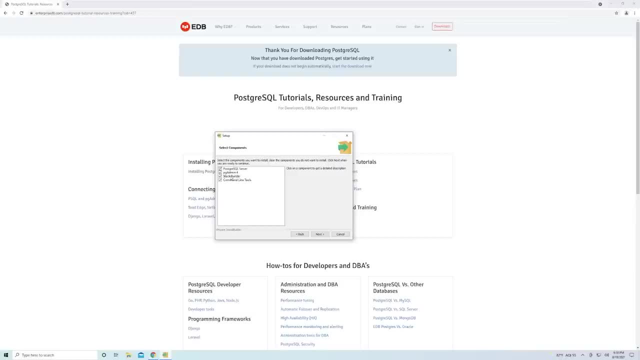 an extra feature that can be used to install extensions and extra features within Postgres. we're not going to be installing any of those extensions, So there's no need to have stack builder. However, it's not going to break anything if you do. leave it checked And then we'll. we won't be using any command line tools to manage Postgres. However, go ahead and just leave that check, just in case you know down the road you actually do want to use it. 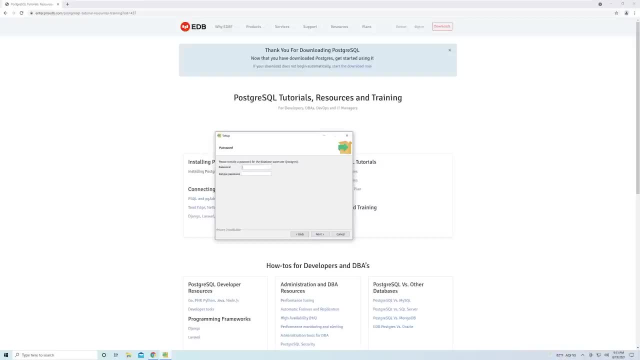 All right, and then once again leave the default data directory. then you have to pass in the password for the super user, So make sure you remember this password. Then you got to specify the port that you want your database to be listening on. The default Postgres port is going to be 5432. You can change it if you want, but you have to make sure that you update everything else. When it comes to creating a code to update that port number, I'm going to leave it as default, as do most people, And then just hit next on this window and then next here, next, and then it's going to start the installation process. 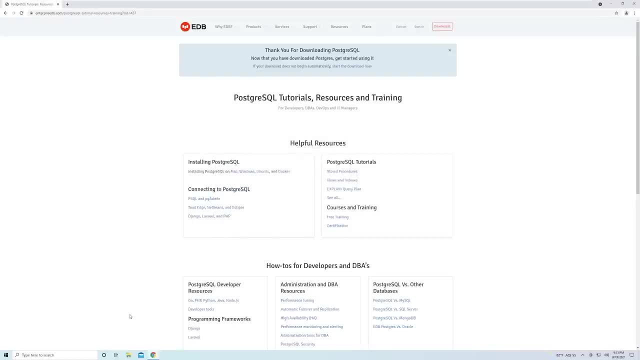 And once that's complete, just hit finish. And, like I said, we're going to be using the PG admin GUI software to manage our Postgres instance. So if you just search for PG admin, you'll see that it's right there, just like that and open it up, And then at that point in the next video we'll start taking a look at how we can use that to not only create individual database instances but also create tables and things like that. 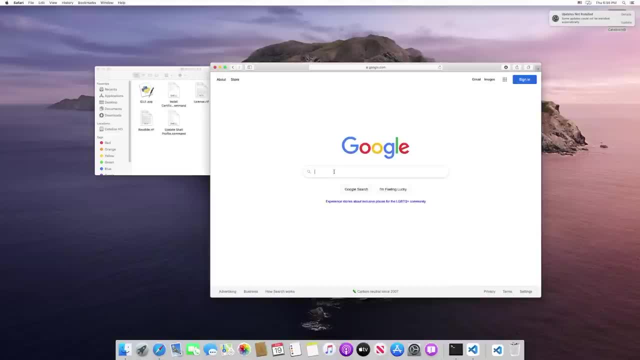 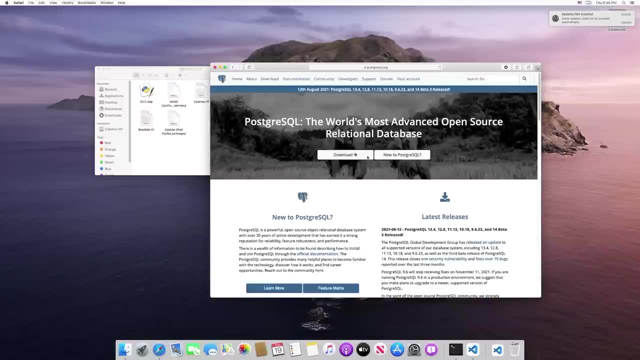 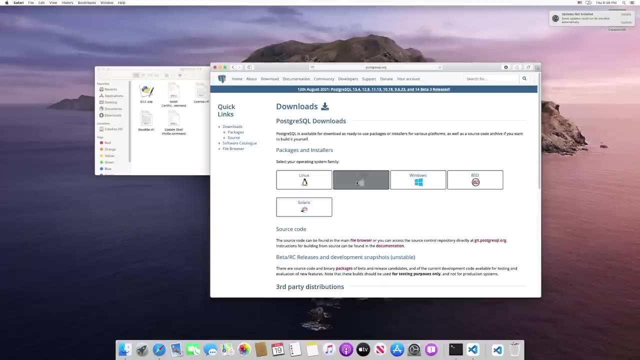 In this video, we'll take a look at how we can install Postgres on a Mac machine. So let's search for Postgres in Google And the first result should be the one that we're looking for And within the Postgres website, just like the downloads button, And this is going to show you the different platforms that support. So we're going to install this for Mac. 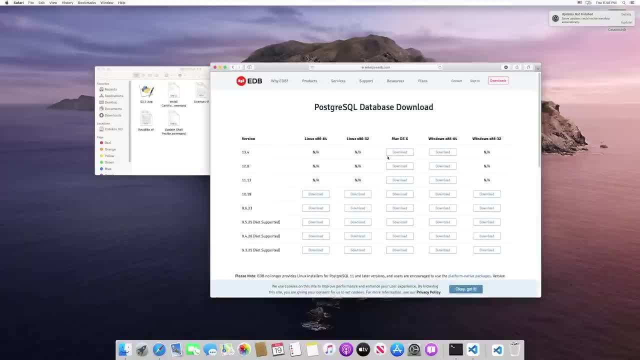 And then select download the installer, And then here we can see all of the versions that we can download. we're going to download whatever the latest version is, So in my case it's 13.4.. If you're watching this video in the future, it's probably going to be some other version, but it should all be relatively the same. So we'll just download under Mac. 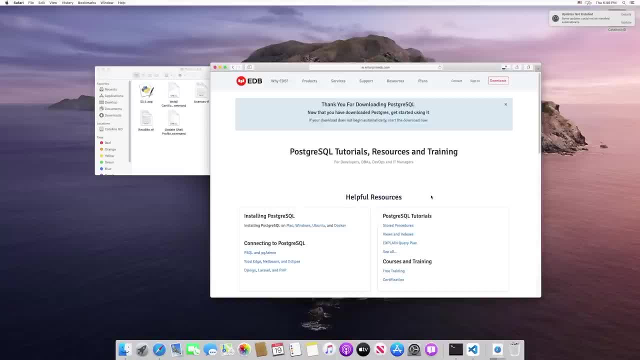 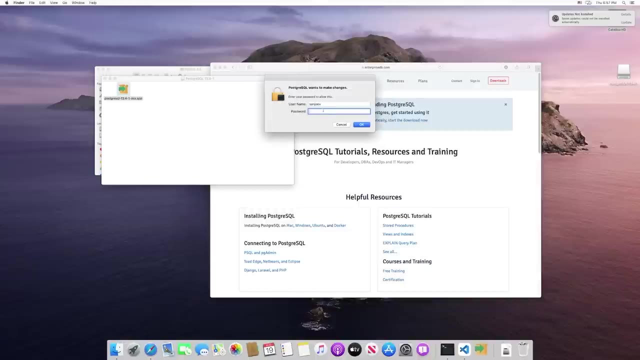 And then we'll click on download Alright and once it's finished downloading, just go ahead and select the DMG file that you downloaded And then we'll set up the installer. And if you get this popup, just select open And then specify your password. 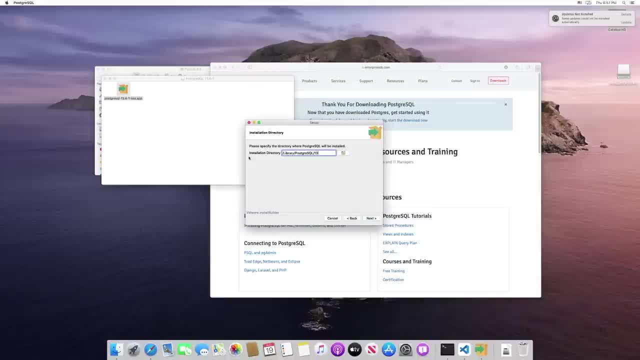 With the installer window open, select next. leave the default installation directory. Now within here, by default, it's going to install four different devices: components. I'm going to walk you through what each of these components does. The first one is: 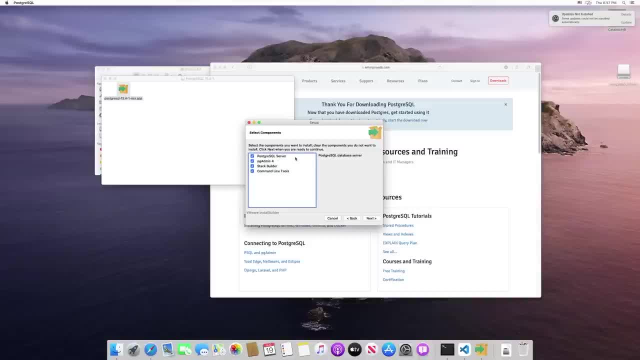 the Postgres server. So this is the actual Postgres database. So we definitely want to install that. Below that is PG admin. This is a GUI that can be used to manage your Postgres databases. We're definitely going to install that, because that's what we're going to use in this course. 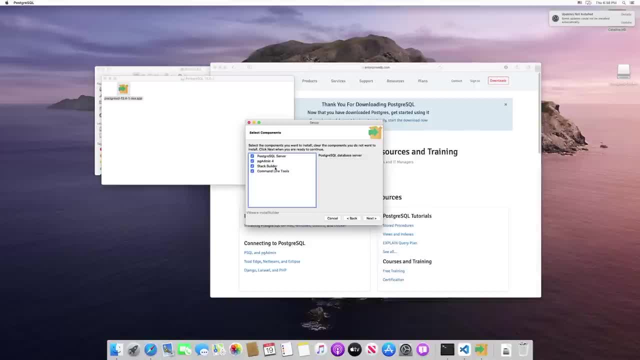 to actually manage our database. Stack builder is an extra- almost like an extra installer that's used to install extra extensions that give Postgres some extra functionality. We're not going to use any of those extensions, So go ahead and uncheck stack builder. And the last one is: 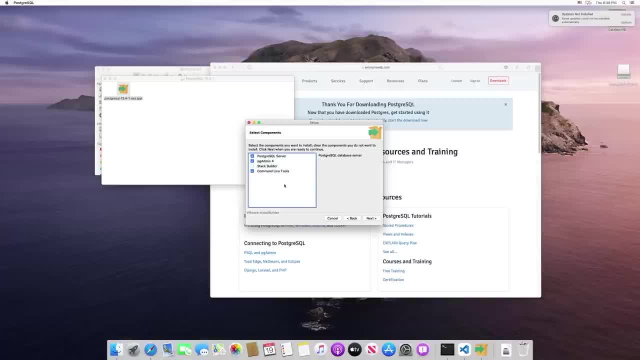 command line tools, So we can manage Postgres through the GUI as well as the command line. In this course we're going to stick exclusively to the GUI. However, I would still recommend downloading the command line tools, just in case you ever do want to use them. 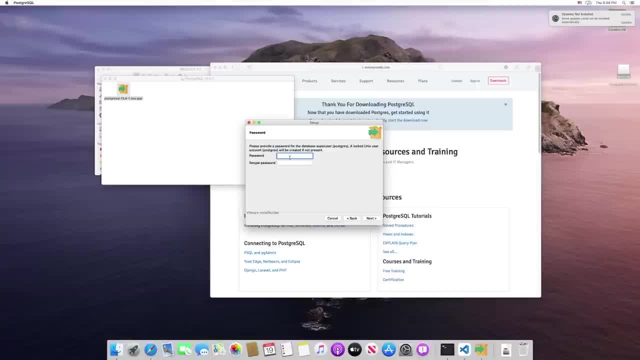 And then specify the default data directory. that's fine. Then you want to give the password to your Postgres instance. So this is kind of like the request, And then you want to give the password to your Postgres instance. So this is kind of like the. 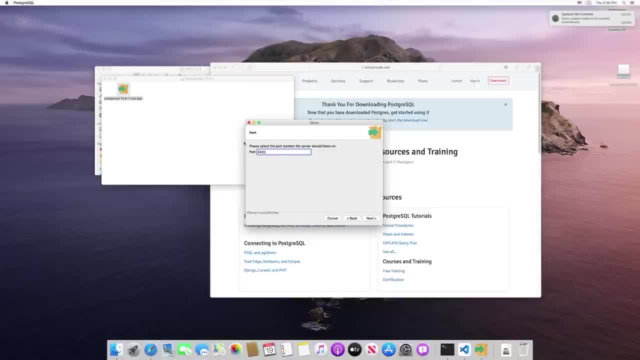 root user equivalent. Here we specify what port we want our Postgres instance to run. This is the default Postgres port. If you want to change it, you can do it, But just make sure that you know whenever we get to actually coding out our API and specifying what port we connect to the Postgres. 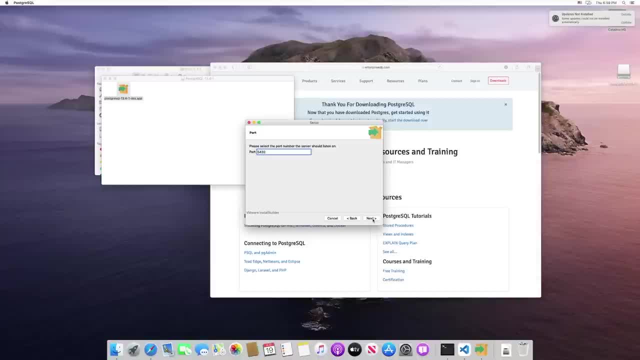 database. make sure you update those accordingly. However, I recommend just keeping it as the default And then everything else. just keep hitting next And then it'll start the installation. All right, and once that's complete, just like finish, it's going to be at that point. 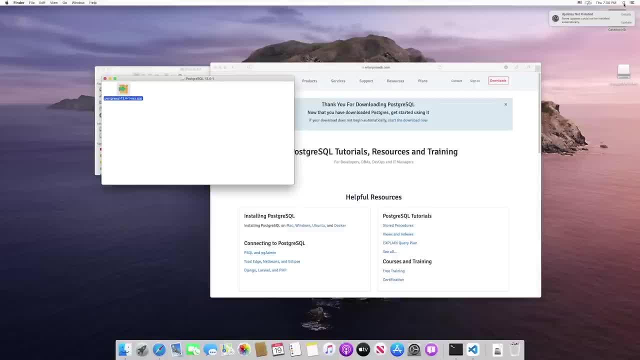 Postgres has been successfully installed, then what you want to do is just hit the little search icon. I want you to search for PG admin. All right, and so if you want to open up PG admin- which we'll cover in the either the next lecture or the lecture after that- just search for it. 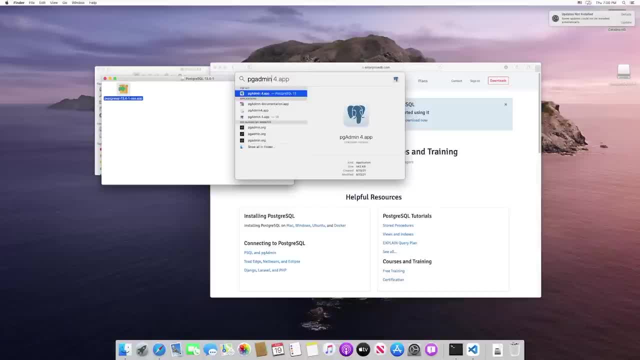 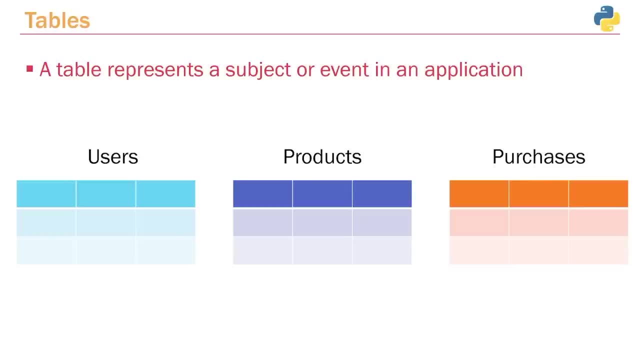 select it, and that's going to open up the GUI tool used to manage your database. Before we get started with configuring our Postgres database, there are a few things that we need to cover, And one of those things is the concept of tables, And this is a very important concept when it comes to working with 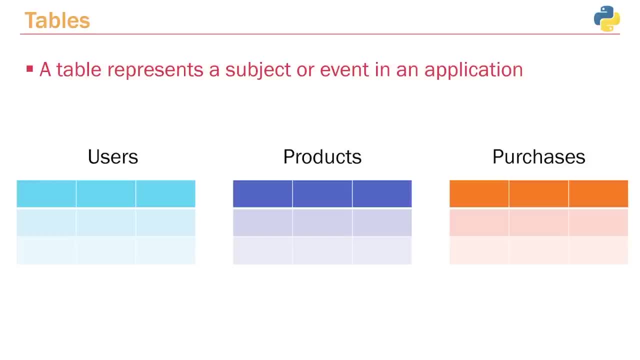 relational databases. So a table represents a subject or event in an application. And so what exactly does that mean? Let's use a example. Let's say we're building out a e commerce application. you're going to have a table that represents each part of your application. So you're going to have 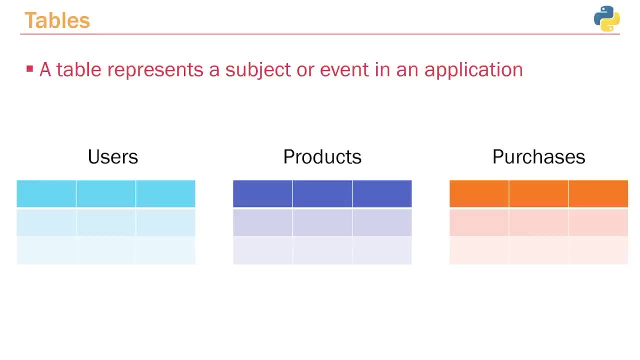 a table for all of the users that have registered. you're going to have a table for all of the different products that you will plan to sell on your website, And then you can have a table for things like purchases and reviews. So each table represents a different subject or event in an 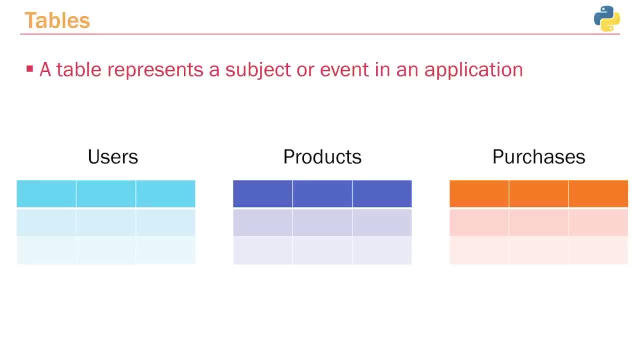 application, And what's amazing about these tables is that all of these tables are going to form some sort of relationship. That's why it's referred to as a relational database And, if you think about it right, the tables that we have listed right here, they're all going to have a very basic and 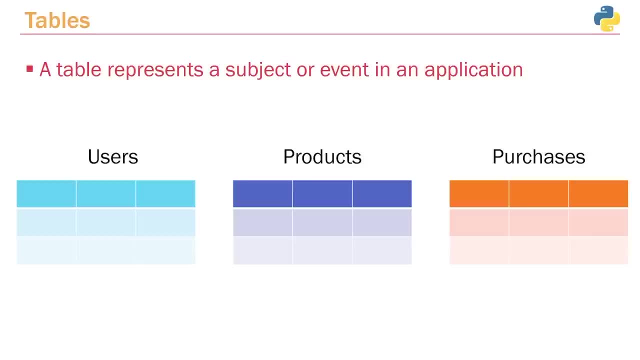 obvious relationship: Right purchases right. when a user purchases something, they're going to have a little bit more of a relationship, is that automatically implies a relationship, because every purchase order has to be associated with the user account that actually filed that purchase order. And a purchase order is going to have a list of products that the user wants to buy. So we 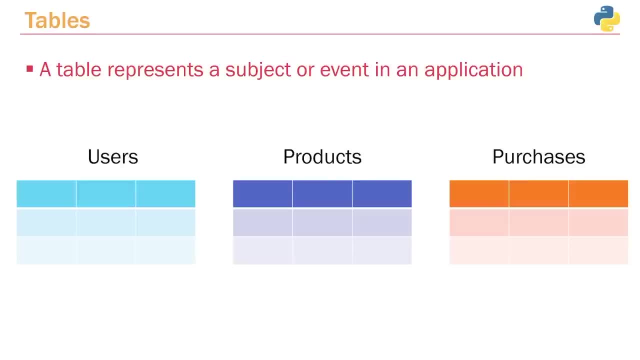 could see right there all of the tables that we have already formed some sort of relationship And it's really important that when you design your database that you figure out what are these relationships beforehand so that you can design a very efficient database Right, just like if we're. 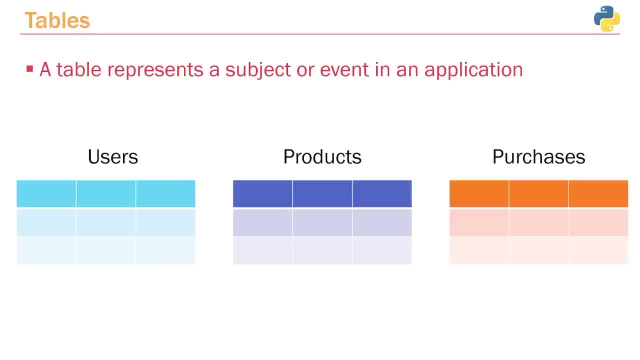 We know we're going to have a table for users. We're going to have a table for posts as well, And we already know that there's going to be a relationship between the two, because every post has to be associated with a user, because users create posts. 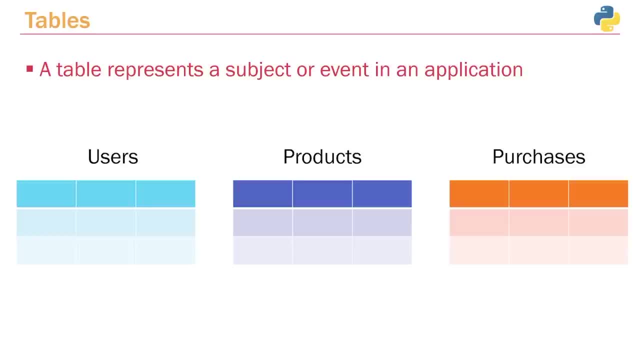 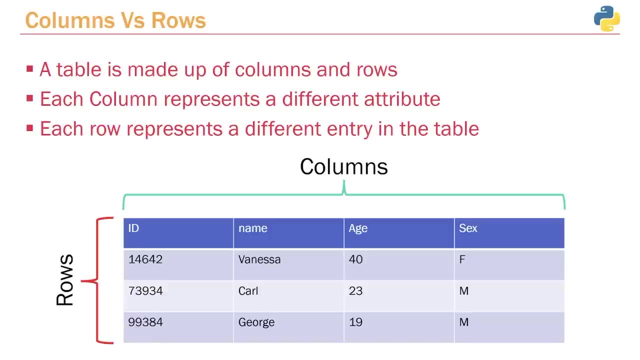 So you can see that. you know, all data has some sort of relationship with one another. Now, when it comes to tables, we have columns and we have rows. A column represents a different attribute, And so if we're building out a table for users, we would create a column for the name. 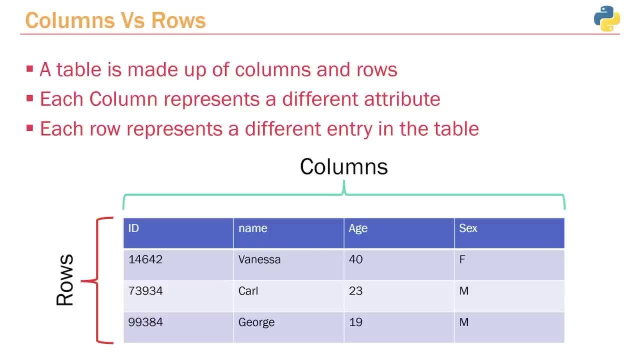 So this column represents the name of the user. We might create a column for their age, their gender. You might create another column for the email that they use to sign up. You might have a column for their billing or shipping address. It's up to you to figure out what are the different attributes we need to model a specific user. 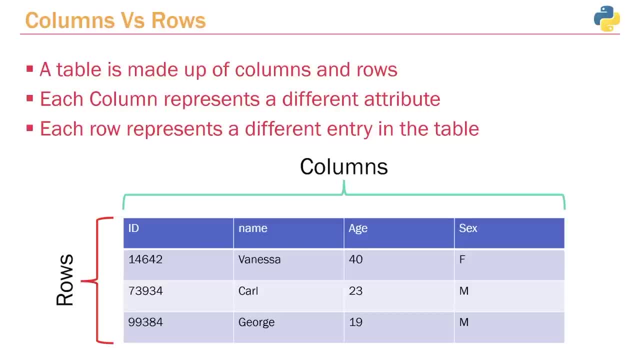 Then we have rows. Rows are very simple. Each row represents a different entry in the table. So we have a user's table. Then each row represents a unique user. So row one: this is the user Vanessa. Row two is going to be the user Carl. 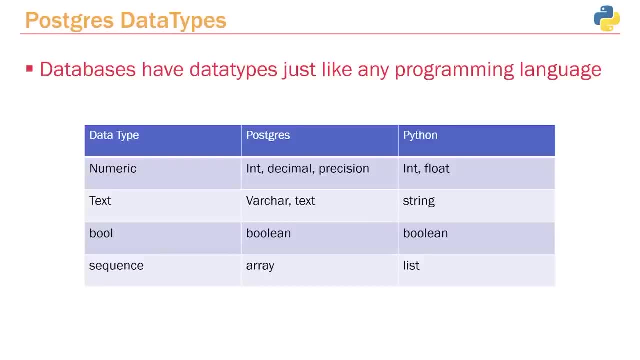 So each row just represents a different entry within the table. Now, databases have data types, just like any programming language, And the reason why this is important is that when you create a column within a table, you need to specify what kind of data type you want to use. 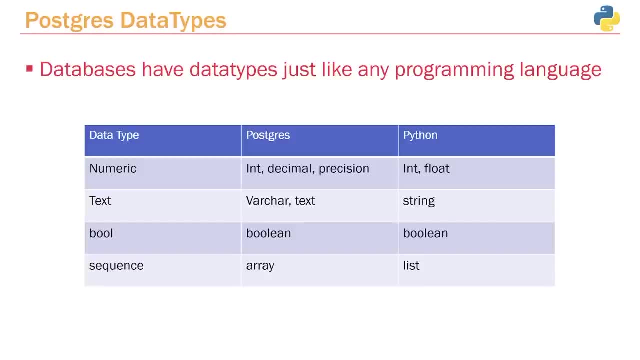 And that decision is going to be ultimately based off of what attribute this column represents. And so we have data types, Just like any other programming language, like Python. And so if we were building out a table for, you know, social media posts. 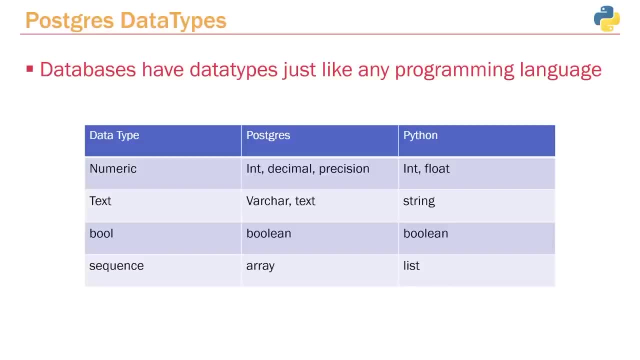 one of the things that we might have is a column for what are the total number of likes or retweets, And so for something like that, you would want some sort of data type that's numeric, You know, a data type that models numbers. 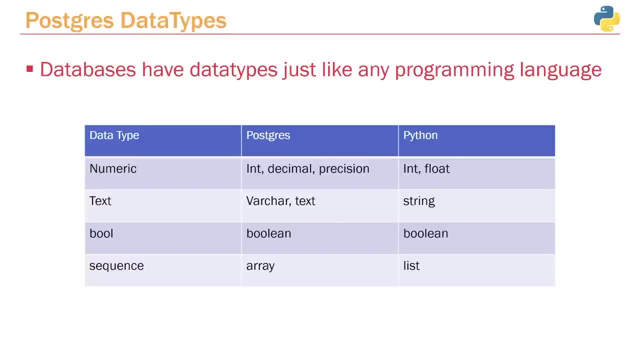 And in Python, you know, we have two main data types: We have integers and we have floats, Integers being whole numbers, floats giving you decimals. Well, Postgres has the same thing, right: It's going to have integers. 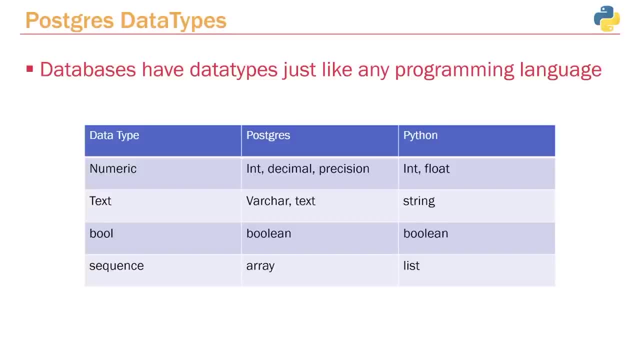 It's going to have decimals and a few others. Keep in mind that you don't need to worry too much about that. Just understand that there are numeric data types within Postgres that are just like Python. So when it comes to the number of likes of Postgres, you know. 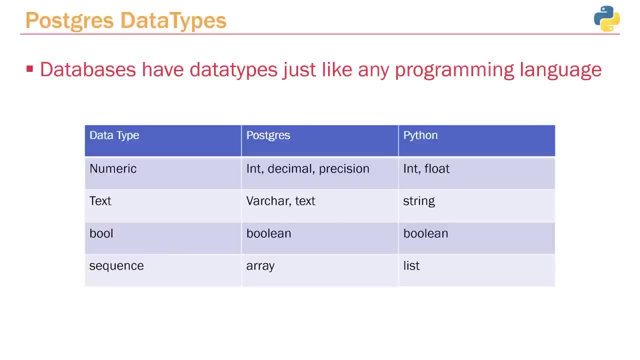 maybe we would use something like an integer, because we're not going to have a half, a like or anything like that. Then, if you're trying to model, you know someone's name or email or address. right, we would use some form of text. 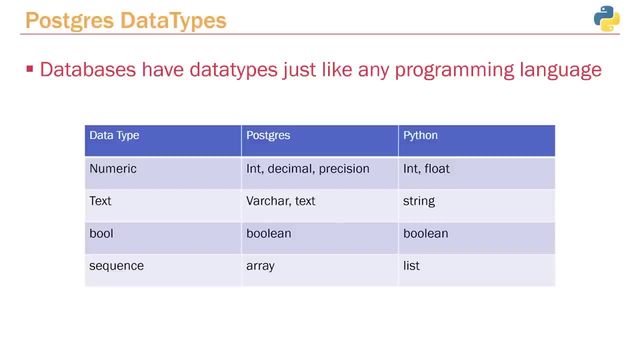 And within Python or any programming language, you have strings that allow you to to represent text. within Postgres, We have the same thing, It's just called something different. We have a Varchar, which is just short for varying character, which is once again just a string. fundamentally, 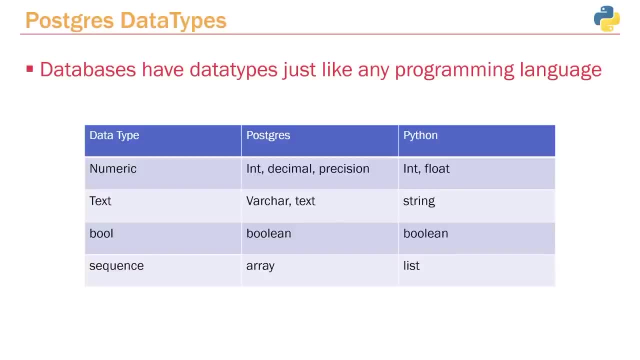 And then we have text right. They're both going to do the same thing. Don't worry too much about the differences. Just understand that Postgres does allow you to work with text just like any other programming language. It's just called something different. 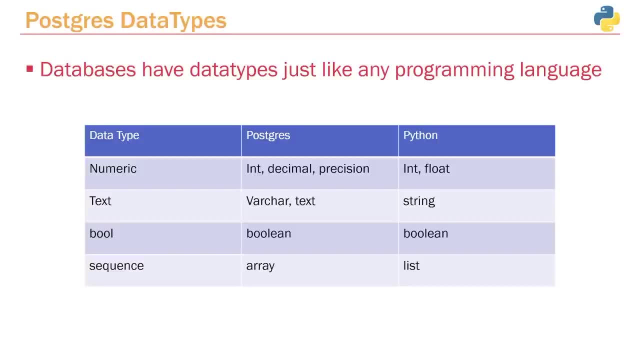 And then for Booleans, Postgres and Python- they both support Booleans- They're going to work the same way. It's either true or false, Very simple. And then within Python, you have a string that's going to do the same thing. 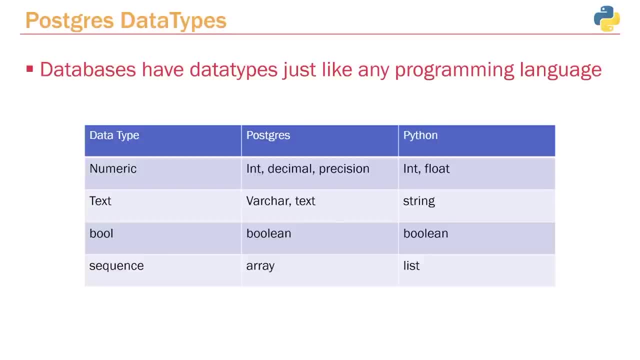 It's just called something different. And then within Python we have lists. So anytime you want to model, you know multiple instances, so a list of something. we have arrays within Postgres And you'll see that when you work with relational databases you'll see that arrays aren't used very. 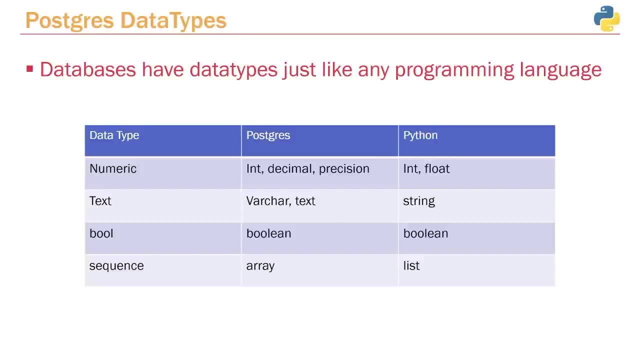 very much, because a lot of times if you're using an array, it may be better to take that column and just convert it into its own table. But, like, like I said, you know, don't worry too much about that, We'll go over that in some upcoming, upcoming lectures. 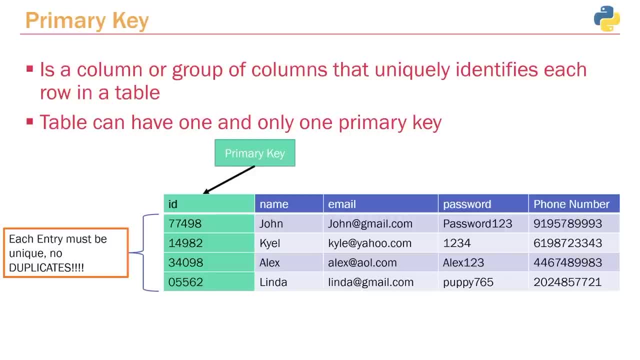 When we create a table, we have to specify something called a program. We have to specify something called a primary key, and a primary key is a column or a group of columns that uniquely identifies each row in a table. So what exactly does that mean? 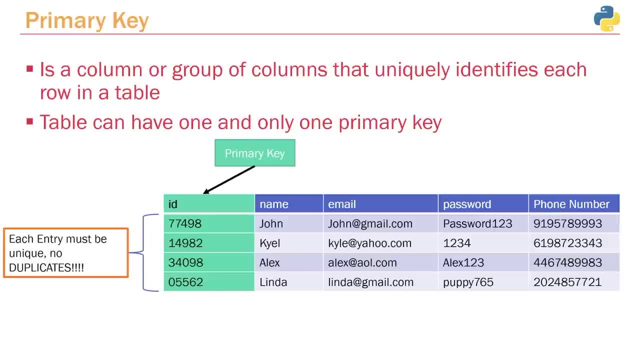 Well, we need to tell Postgres essentially how can we uniquely identify each entry in our table, each row, And so we have to give it a special column that ensures that every entry for that specific column is unique, And keep in mind that we can only have one primary key per table. 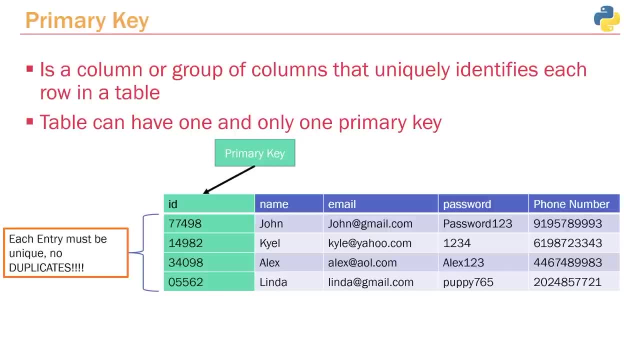 You can't have more than one. However, a primary key can span multiple columns. However, let's keep Things simple for now and just assume that primary keys are really just one column, And so a lot of times when you create a table, what we have is a column for a unique identifier. 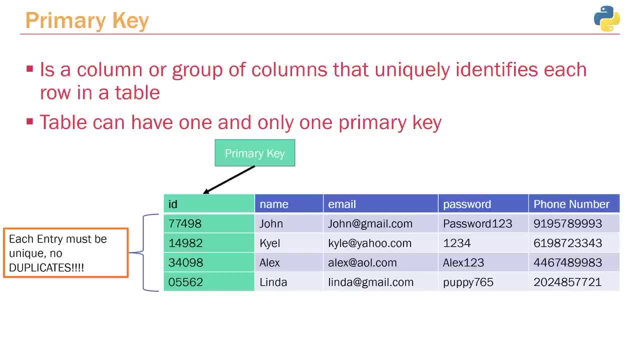 So anytime you create a new user, usually you're going to have an ID associated with that account and that ID is going to be unique, And so the ID associated with John is going to be 77498.. And that's how we uniquely identify each user based off of that ID. 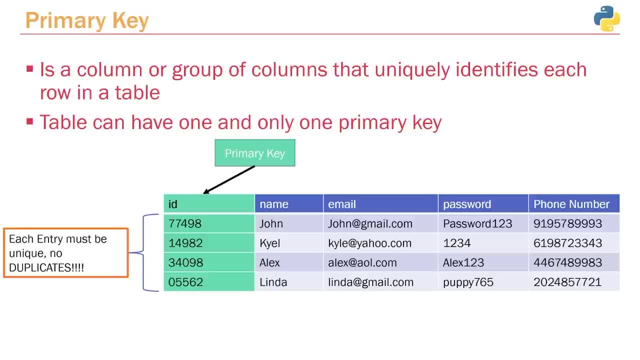 And so it makes sense to select that as the primary key, Because we Already know that each ID is going to be unique, So it fits the perfect definition of what a primary key is right, And so the only requirement for something to be a primary is that each entry must be unique. 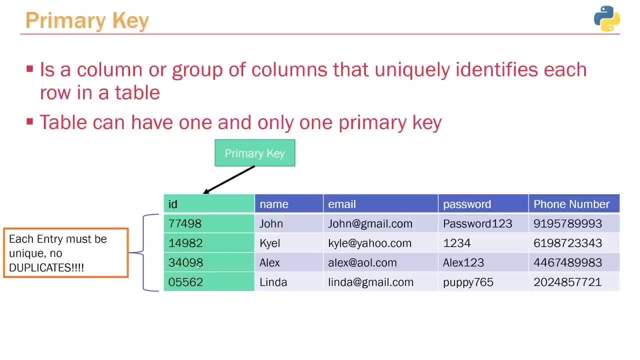 No duplicates. We can't have the same ID for another user, And so you're probably thinking at this point that, Hey, we're going to create an ID column for every table and then make that the primary key. I'm going to tell you that that's not quite correct. 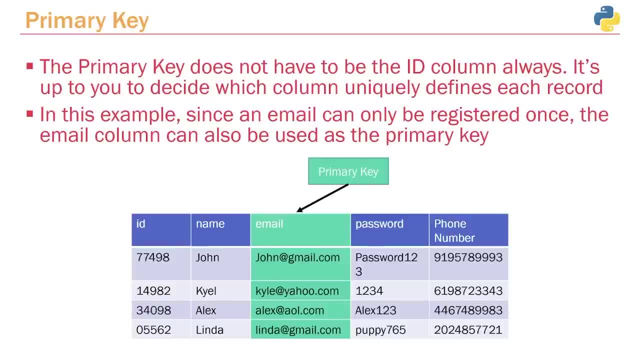 The primary key doesn't have to be the ID column always. In fact, your table doesn't even have to have an ID column. It's up to you to decide if you actually want to have that. There are certain instances where you may not want an ID column. 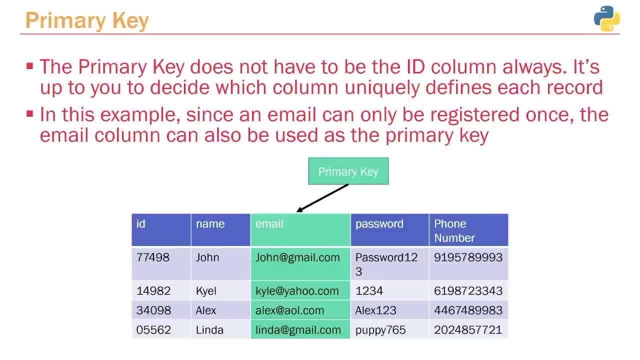 And so if you don't want to use the ID column, or if you don't have an ID column, you need to ensure that you have some column that's able to uniquely identify each and every entry. And so one good example of that- when sticking to the users table example- is that generally in an application, a user can only sign up with an email once. 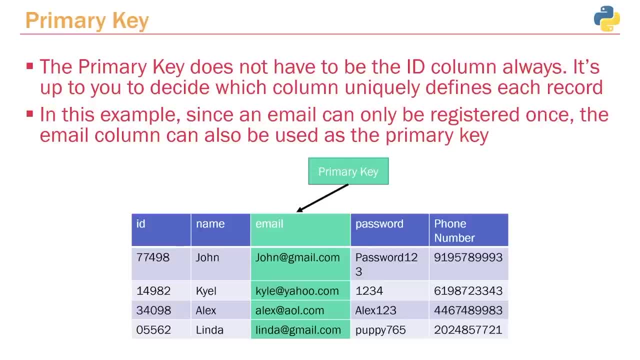 So we know that an email is always going to be associated uniquely with one account, right? We can't have two users with this, The same exact email. that's not going to work. That's usually not allowed. So we could definitely use our email column as a primary key. 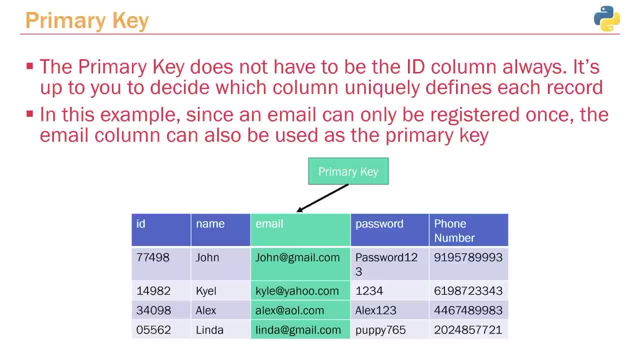 But there's plenty of other examples. right Phone numbers, right. Generally, I can't sign up with the same phone number for two different accounts, So we know phone numbers are going to be unique for the guys that are in the United States. 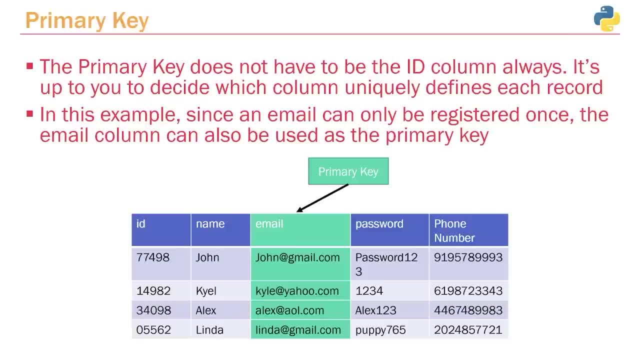 You know what a social security number is. Two people can't have the same exact social security number, And so there's a lot of different things that you can use to choose for the primary key. Uh, just Keep in mind it's not always the idea. 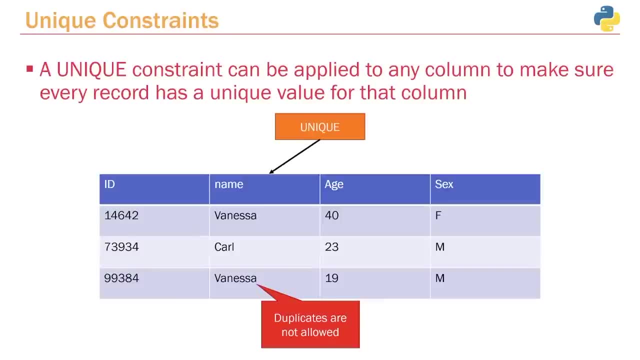 So that's the main thing I wanted to focus on in this slide. Now, as we go through creating our table uh and creating each of the individual columns that represent a certain attribute for that table uh, we can add in extra constraints for each column so we can put in extra little conditions. 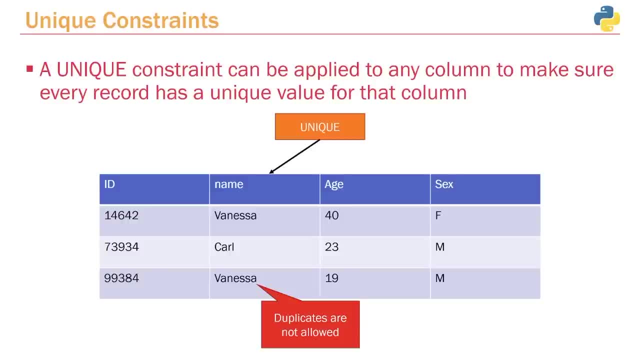 And so we already talked about the column. that's going to be the primary key, and we know that the primary key has to be unique for each and every row. But what happens if we have another column That Isn't the primary key? but we want to ensure that each and every entry has a unique value for that specific column, right? 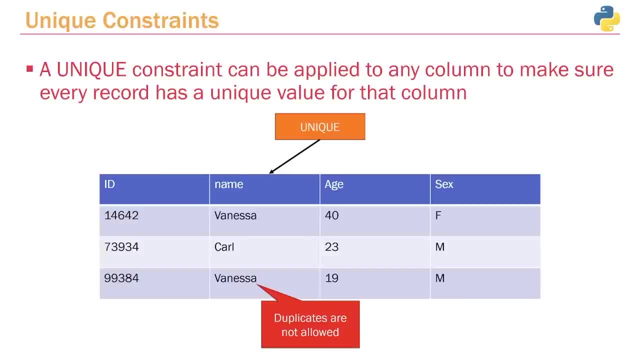 So take a look at the name column in this case. Let's say that we we won't allow two users to share the same exact name. Is there any way we can tell Postgres to perform that check for us? Well, we can add in what's called a unique constraint. 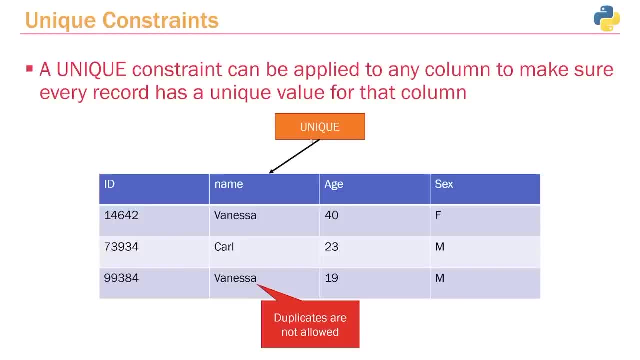 So we can, when we create the table, say that I want to make this column unique by adding the unique constraint, And so that way, anytime I add in a new user, it's going to check the name and it's going to check to make. 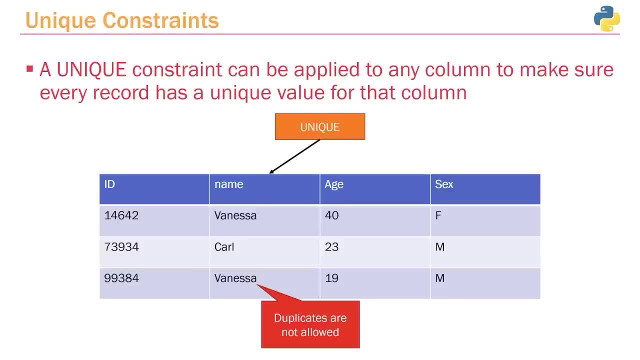 Sure that there's no other users with the same exact name And if there is, it's going to throw an error and we can do this with any column. You can do it with all your columns if you wanted to. That's not necessarily something you're going to do, but I just want to make sure you guys understand that. you know we can perform extra checks for each entry by adding in a constraint. 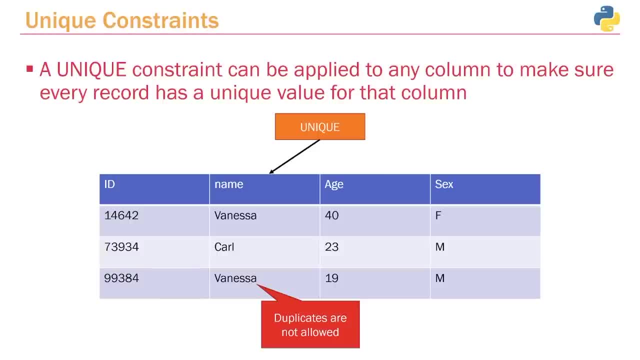 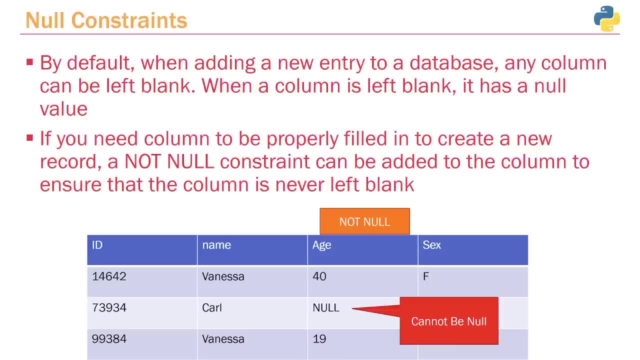 The first constraint that we covered is the unique constraint, but there are plenty more Now. the next constraint is called the null constraint And when it comes to creating columns, by default Postgres allows you to Leave a column blank, essentially so I can add in a new user. 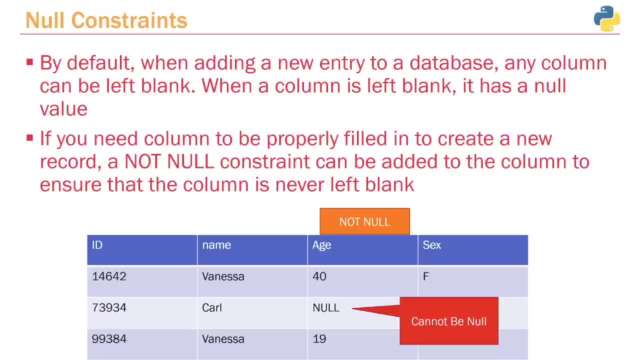 And I can say that I can leave the name column blank. So instead of having Vanessa for the first one, I could just leave it blank and not put any data in. And so what Postgres will do is it'll put in a value of null because we didn't provide it. 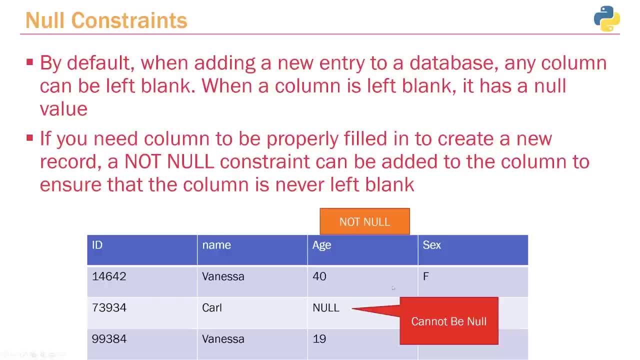 And I could do the same thing for age. I don't have to pass in an age by default, and I don't have to pass in a gender by default as well, And it will put in a null value for each and every one of those. 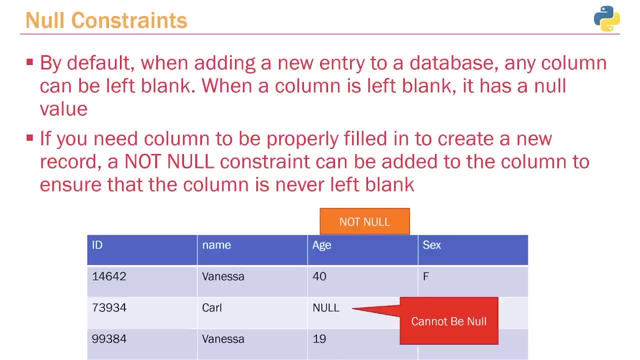 But let's say we want to tell Postgres to perform a check and say, hey, I don't want you to be able to Create a user that doesn't have an age. So what we can do is we can put in a constraint, and this constraint is called a, not null. 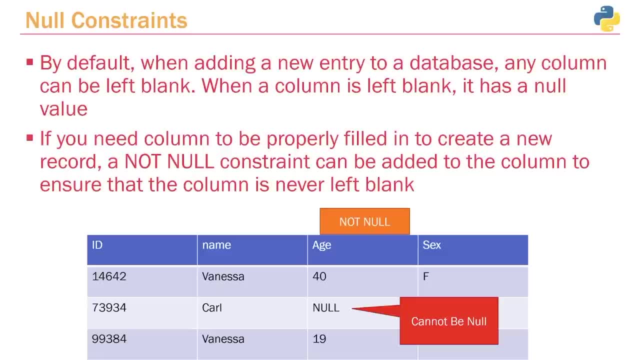 That means we are not going to allow it to be null, right? We are not going to allow Postgres to use a null value. So if we try to add in a new user called Carl and we don't give it an age, Well, Postgres sees that this column is not allowed to be null and it's going to throw an error because it's not null. 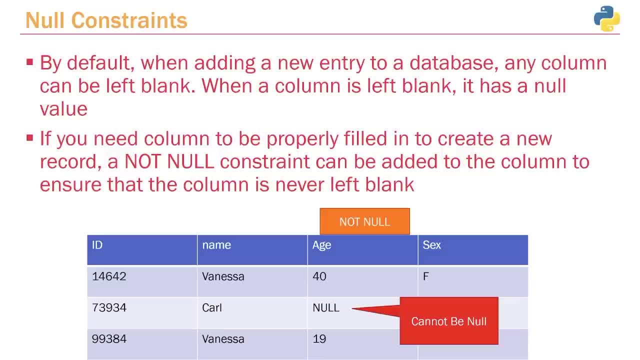 So that's the second constraint, And I think these are the two main things that I want to focus on, And I think at this point We have a good enough understanding of the different things that we can do with tables, columns and rows that we can go ahead and start playing around with Postgres and really digging deep into how tables are created and how they work. 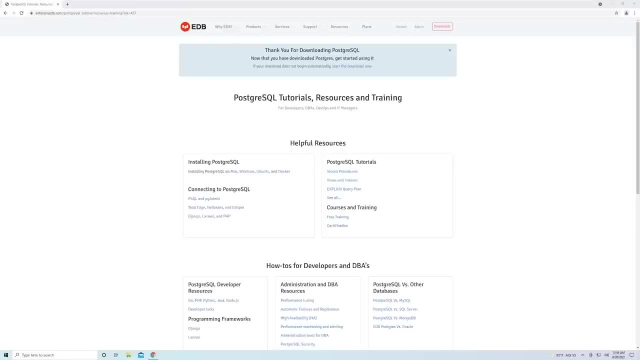 In this video, we'll start taking a look at PG admin, which is the GUI that we use to manage our Postgres instance. We'll take a look at how we can define our tables for Postgres. We'll take a look at how we can create entries in our database, as well as how to modify and delete them as well. 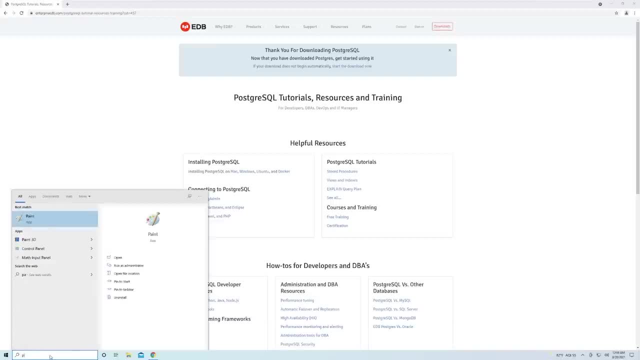 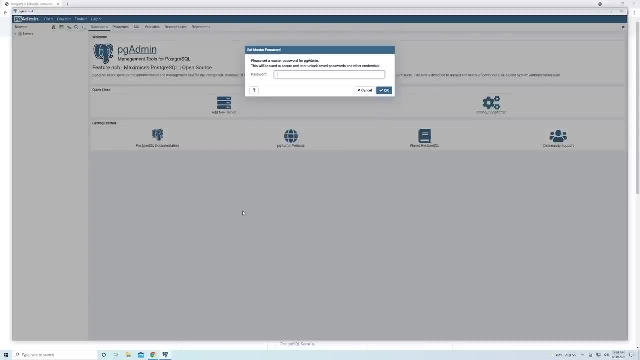 So go ahead and search And you're under your applications for PG admin And you'll see that once it pops up for the first time, it's going to ask you to set the master password for PG admin, And it's important to understand that this password is for the PG admin GUI. 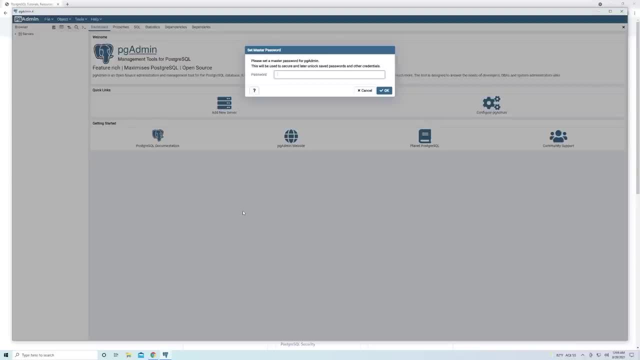 It has nothing to do with the password that you created during the Postgres installation. This is strictly for PG admin itself And the reason to ask for a password is that, ultimately, we can store our passwords for connecting to our different Postgres instances Within. 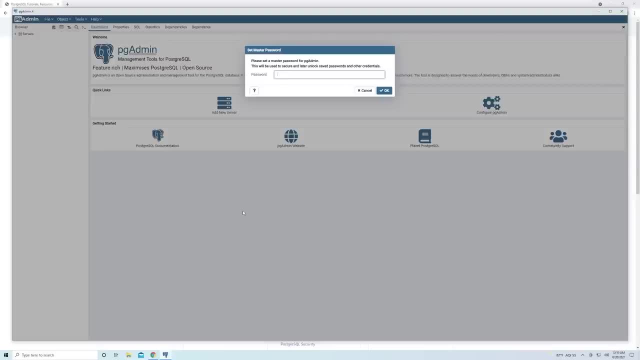 PG admin, so that we don't have to enter it every time we want to connect to our database, And so that's why we have to create a master password, so that we could store all of the individual passwords for all of our Postgres instances. 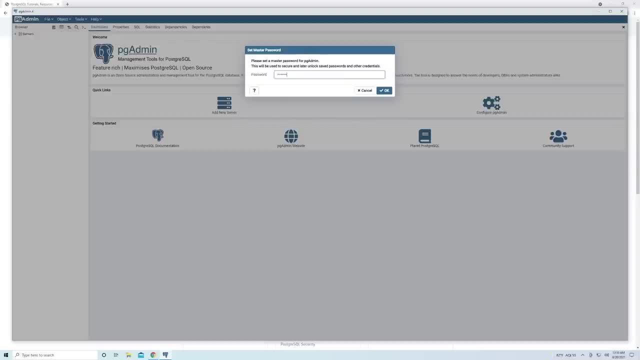 So I'm just going to create a random password in this case, And keep in mind it does not have to match the password that was created for your Postgres instance. These two have nothing to do with one another. Now the first thing that we want to do is specify the connection details for connecting to our Postgres instance. 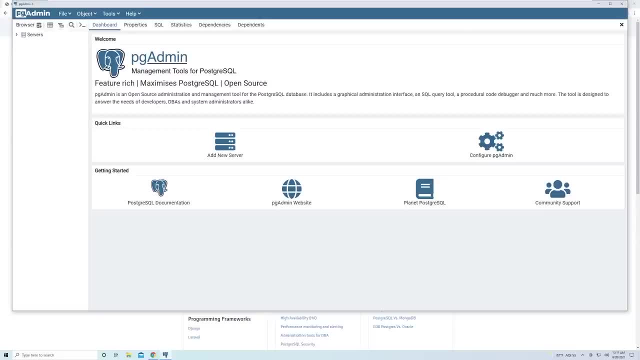 And what's nice about PG admin is that we can It'll remember all of the servers that we've ever connected to, so that we don't have to manually input this information every time we log in. Now, PG admin has done a little bit of the work for us automatically. 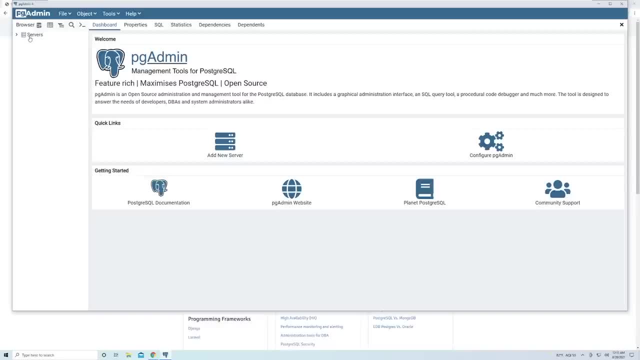 So if you see under the server section- this is where we define our individual Postgres instances- Just hit the little drop down arrow and you'll see that there was a server called Postgres QL 13 already created for us. So by default, when you install Postgres, we know that we're going to have a local Postgres instance running on our local machine. 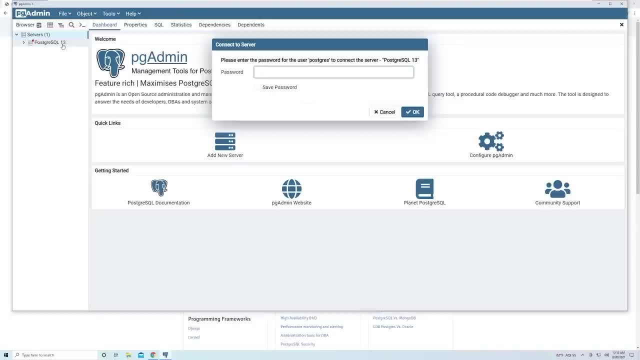 So it's going to Automatically set up the connection details for that instance. The only thing you have to provide is the password for connecting to that instance, And so now we want to pass in the password for the Postgres user for the Postgres instance. 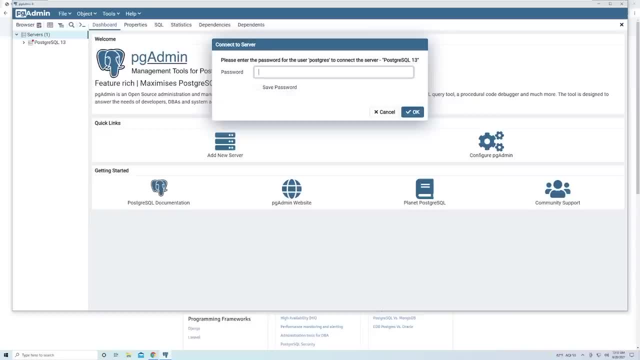 And this password isn't the password that we just created a few seconds ago. This password is the password for Postgres itself, So this is the one we created during the installation process. So go ahead and put that in there, And then you can choose to save this password so that you don't have to reenter it. 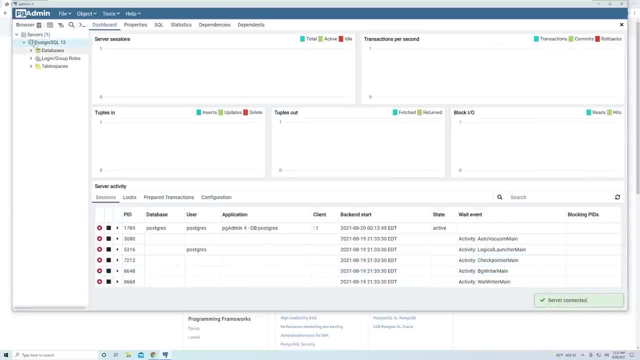 I'm just going to skip that for now. And so now it's taking that password and it's now connected to our local Postgres instance, And so you'll see a little bit of information about Things like you know, what's the sessions, what are the transactions per second? 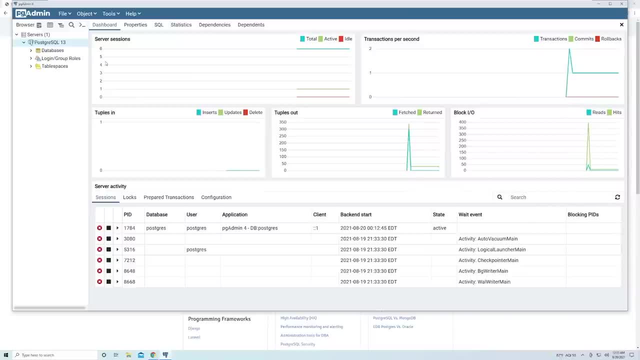 So you'll see it, not a lot of nice little, pretty charts. However, I want to make sure that you guys actually understand how to define a new server instance. So what we're going to do is we're actually going to create this from scratch. 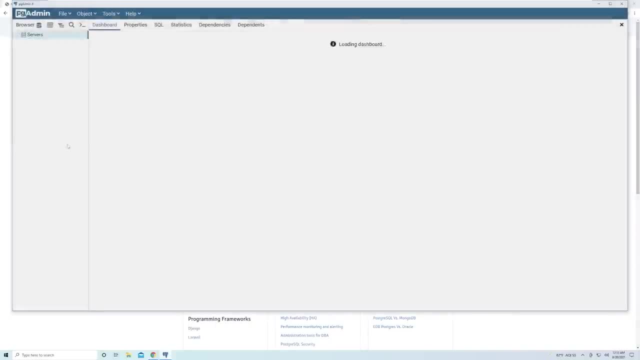 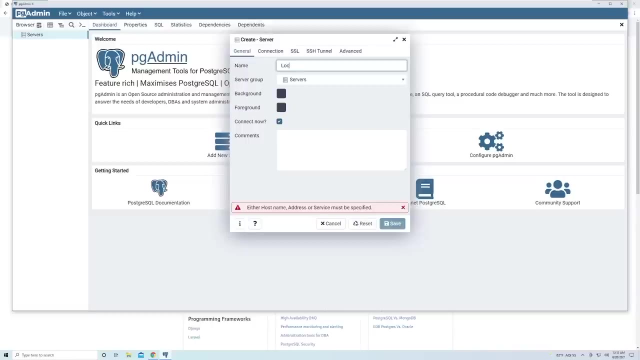 So I'm just going to select this, We're going to select remove server And we're going to do this straight from scratch. So do create server. Let's give this a name. I'm going to call this my local Postgres instance, because that's what it is. 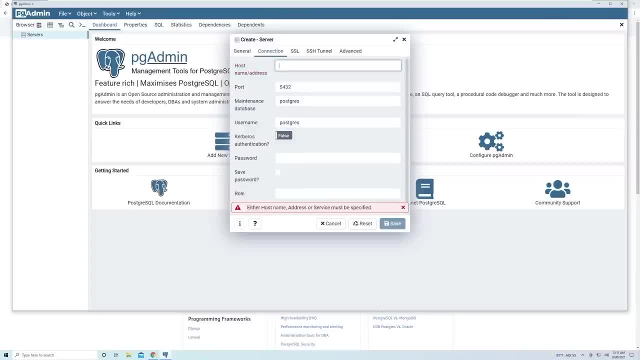 Local Postgres, Then we have to specify the connection details. So here we give the IP address that the Postgres instance runs on. because this is running on our local machine, We can just say local host. However, if this was running within AWS or some cloud provider, that cloud provider would have would provide you a password. 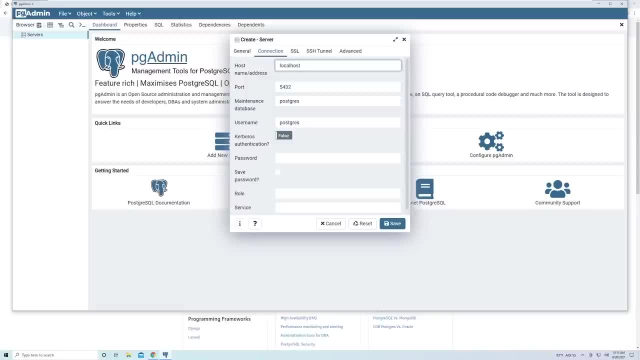 Sorry, an IP address or even a domain name to connect to, And that's what you would specify here in this case. But since we're connecting to our local machine, we just say local host. Then here we give the Postgres password. 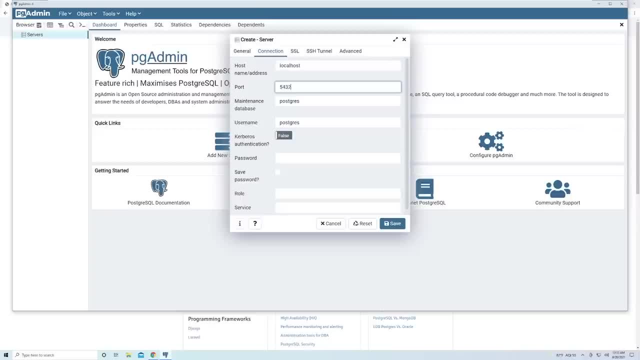 Right when we did the installation for Postgres. we use the default port, So that's why we just leave this as five, four, three, two, And then, as I mentioned, when we connect to Postgres, we always have to give it a, the name of a database to connect to. 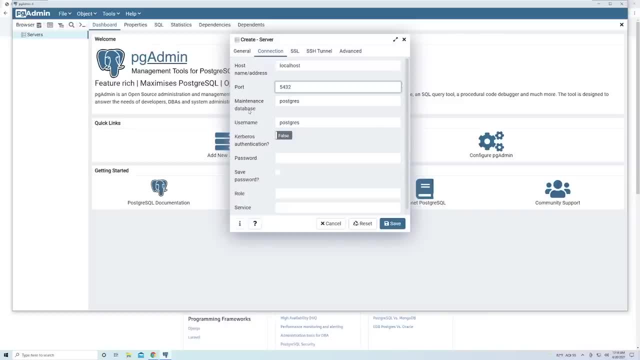 We always have to provide the name of a database to connect to. Since this is a fresh installation, the only database that's going to be there is going to be a database named Postgres, So it's going to connect to that by default. 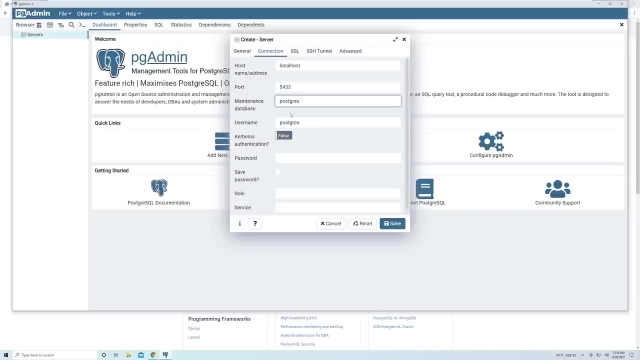 Then we have to give the username and password, and we haven't created A user yet, so there's always one default user. This is a super user, and the username for that user is always Postgres. A little confusing, because the database name is Postgres, the name of the actual DBMS is Postgres and then our username is also Postgres. 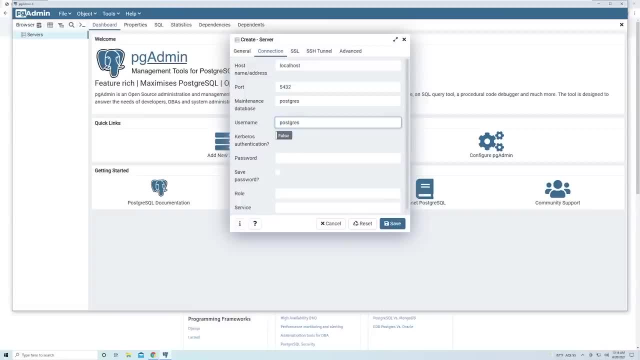 So try not to get all three of those things confused. Then we here we could save in our password. So this is where we put in our Postgres password And then, if you want to save this for a future so that you don't have to enter in every time, you can go ahead and do that. at that point, hit save. 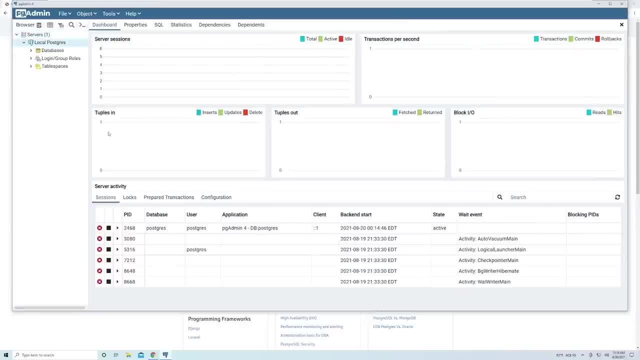 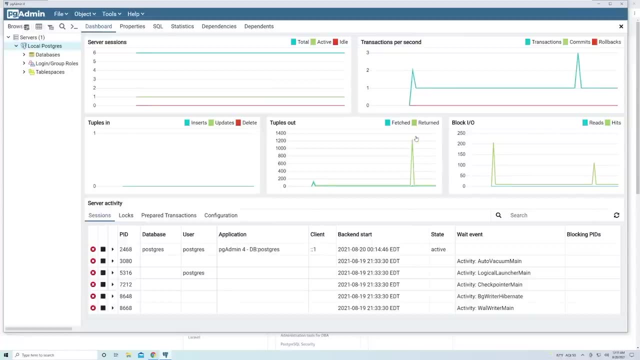 And then you could see That, once again, we created this from scratch. Now, within PG admin, there's going to be a lot of menus, a lot of things that you see and you may be a little overwhelmed, But I want you to keep in mind that a majority of the stuff we won't really even care about. 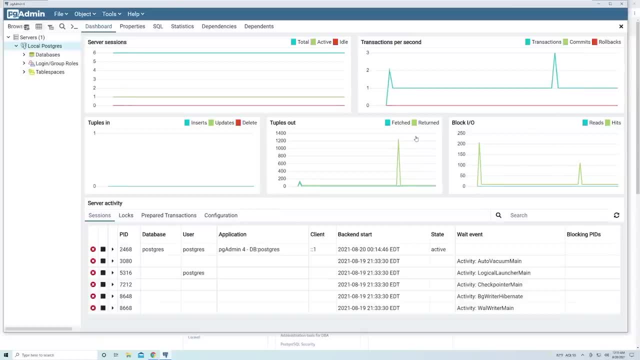 Right. So when you focus on just the things that we care about, you'll see that there aren't many things involved when it comes to PG admin And so, like I said, within a Postgres installation we're going to have individual databases, right, so we can create a separate database for each of our applications. 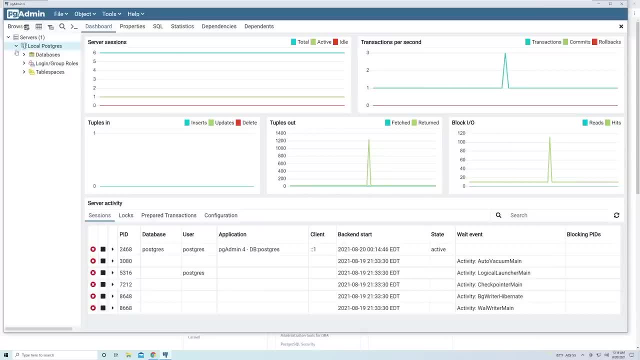 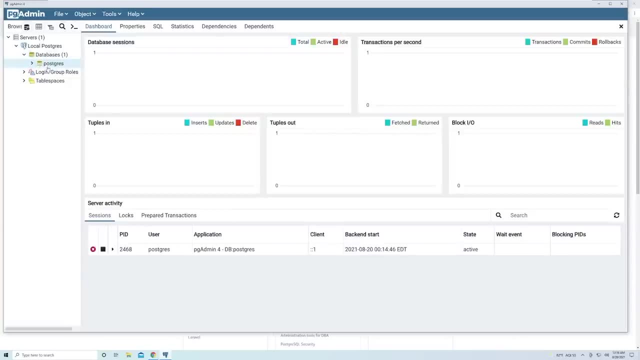 So under our server Right You'll see a section called databases. So this looks a little interesting. Let's click this And then, if we drop this down or expand this, you'll see that we have our one default Postgres instance that was created for us during the installation process. 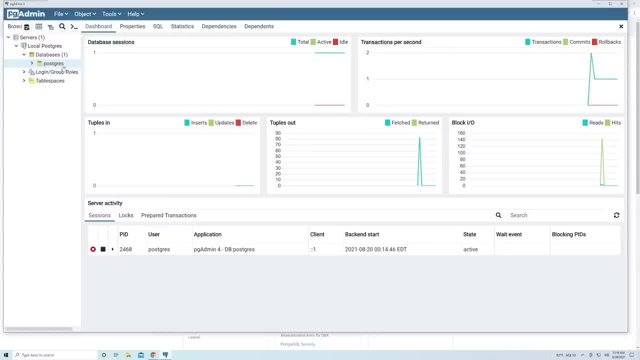 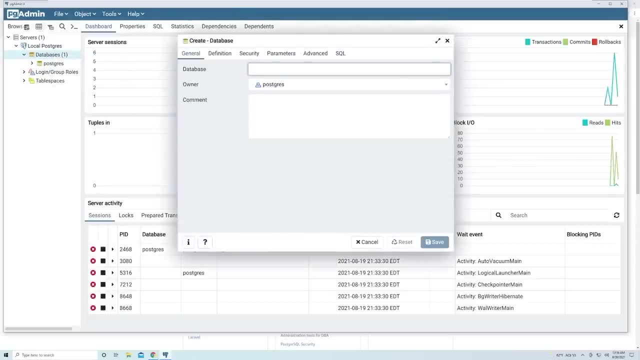 Now we're not going to touch this, We're just going to leave this there. But let's create our own Postgres instance. So right click on databases, hit create and then database. And then here we just want to give the database a name. 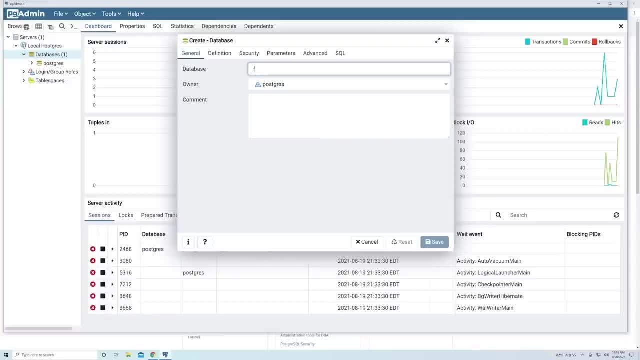 I'm going to call this. I usually just name it after my application name. So since this project is called FastAPI, I'm just going to call this my FastAPI database, And you'll see that there's a couple of other windows. We won't touch any of these. 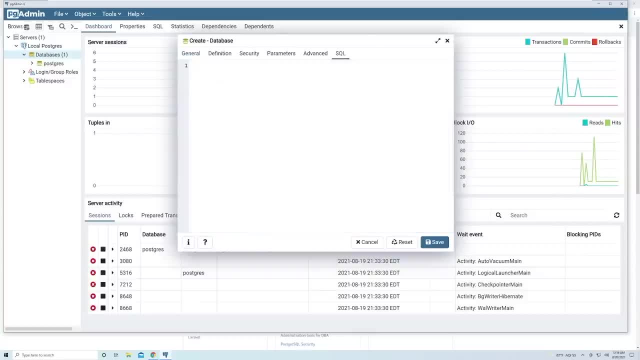 However, go to the last section right here, where it says SQL. And, as I mentioned before, SQL is the language that we use to actually talk to Postgres And, you know, since this GUI is here to manage Postgres, it's going to make our life a little bit easier. 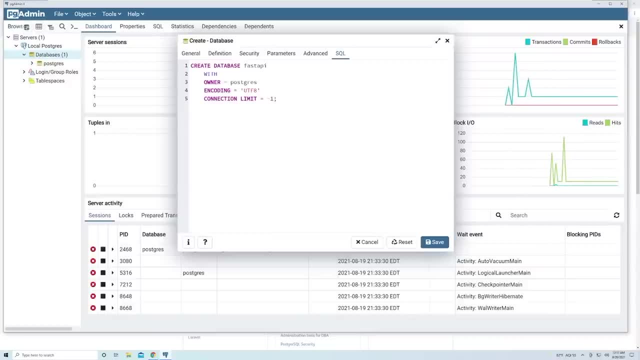 But at the end of the day, it's just passing in SQL statements And so, because we created a database through the GUI, It's kind of abstracting a lot of the SQL away from us. However, what's nice about pgAdmin is it's going to give you the underlying SQL that's used to actually create this database. 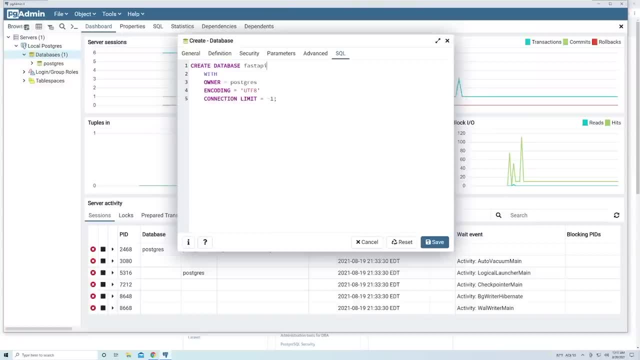 So we could see that it's just a command that says create database and then the name of the database we gave it Here. it's just specifying the owner, the encoding and the connection limit. Technically we could remove all of these lines and just take the semicolon and just put it right here. 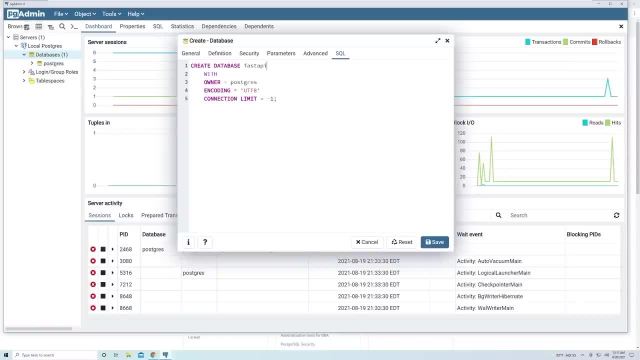 And then we can just do create database FastAPI, and that's how you do it through the command line. I think it's just nice and helpful that it provides this for us. However, ultimately we won't need to do that because we do have pgAdmin, so we can do it all through the GUI. 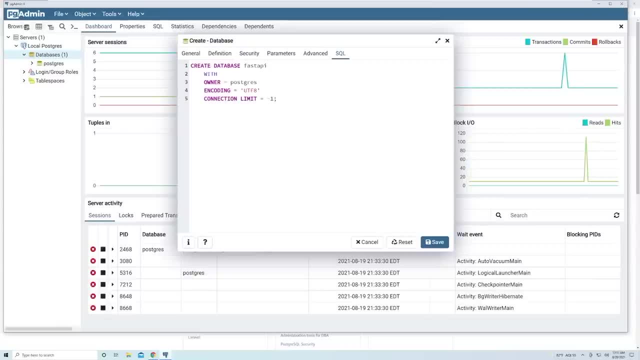 And you know, if you guys are worried that we're not going to cover SQL, believe me we will. But I just want to make sure we start off by, you know, taking a look at the GUI, learning it the easy way. 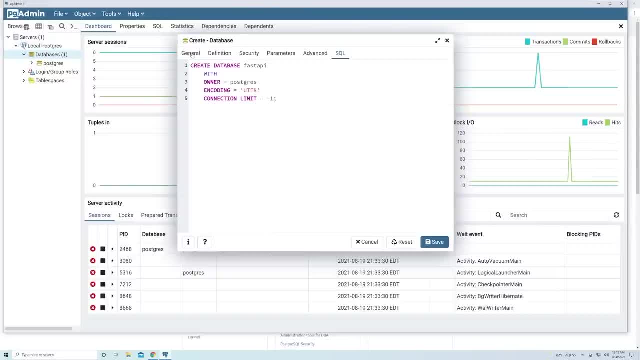 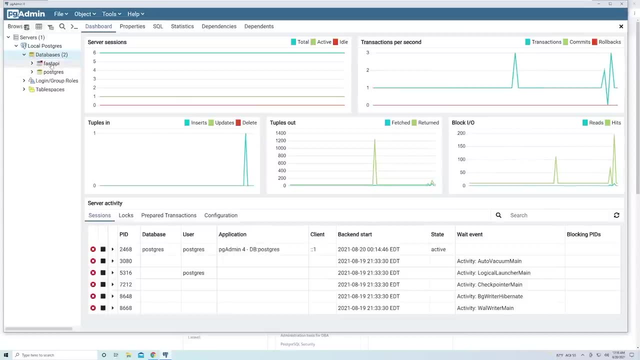 Then we'll learn how to do it the harder and proper way. But once we got this set up, go ahead and hit save And you'll see that we have our new database. right now There's an X, But if as soon as you click on it, 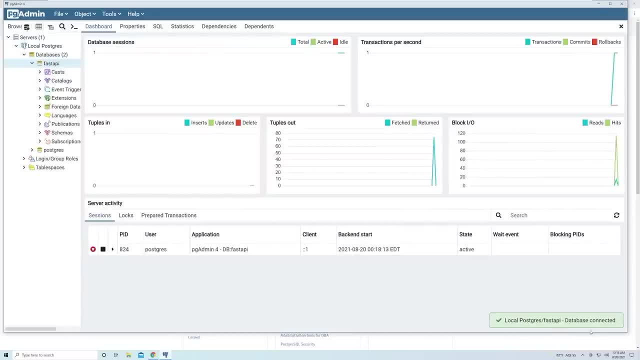 It's going to turn yellow, which means that we have now successfully connected to this database, And then, under this database, you're going to see a lot of different options And, like I said, we're not going to touch most of these. 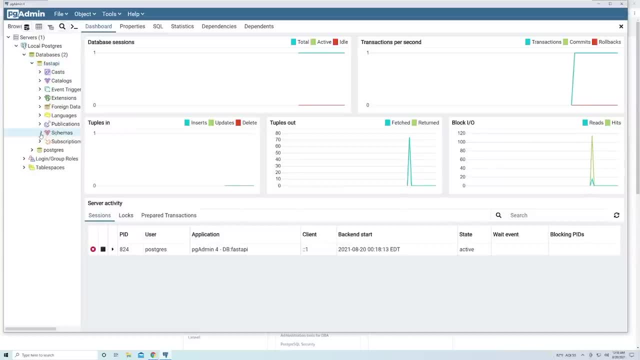 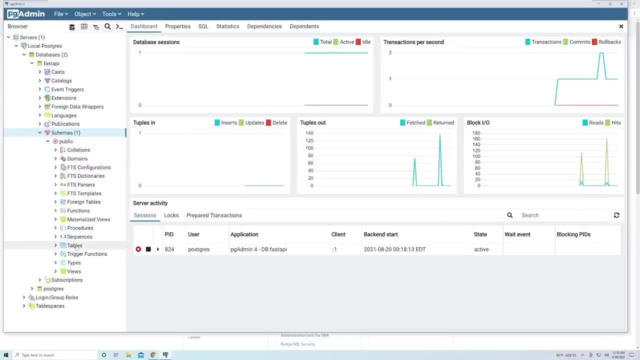 Instead, the only thing that we want to focus on is under schemas. So under schemas and then under public- and I'm going to move this over for you guys- You'll see that there's one important section called tables. So this is where we actually create and define our tables. 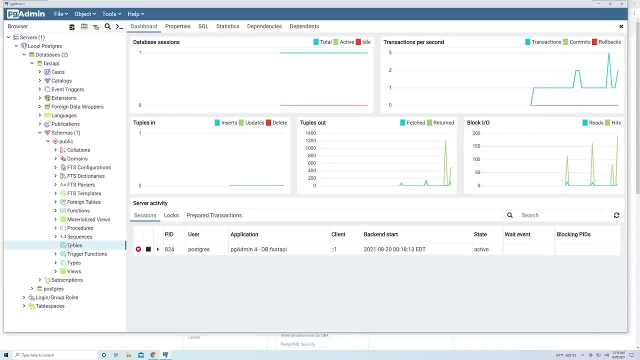 So right click this And actually, if we do it, If we hit the drop down, you see there's no tables. but that's to be expected because this is a brand new database And let's go ahead and create our first table. 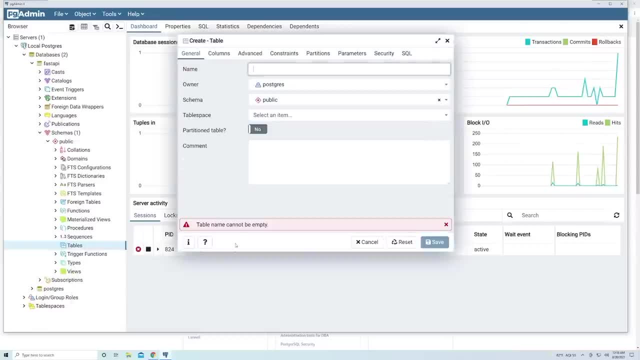 So we'll do a right click, create and then table, And then let's give this, our table, a name. So let's say we're sticking with the whole e-commerce example, So we're going to create a table called products. So this table represents the different products that we're going to sell. 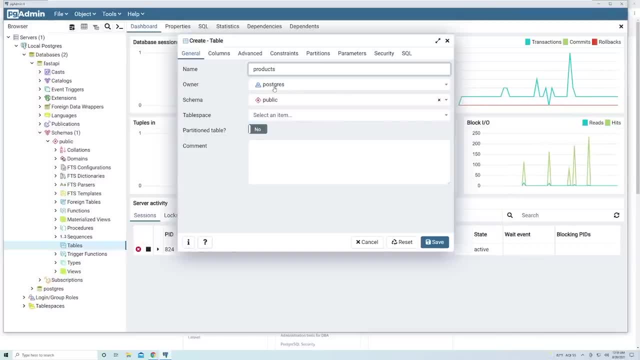 Don't worry about any of these other fields. It says the owner is Postgres because we're logged in as the Postgres user. However, you know, if we log in as a separate user, Then you would see the owner get updated accordingly. 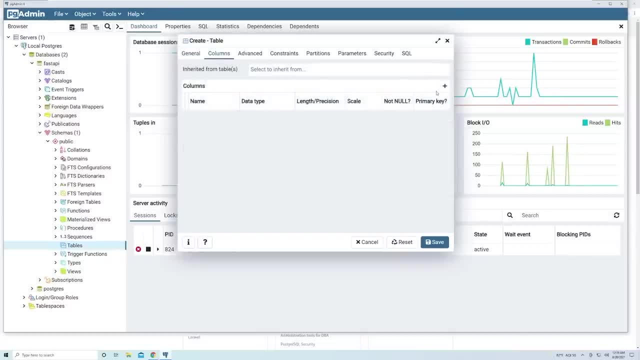 If we go into the column section, this is where we define our column, So this is where we're defining what is referred to as the schema of the database. So to add a new column, just hit the plus icon, And so now the first thing that we need to do is: let's figure out: what attributes does a product need? 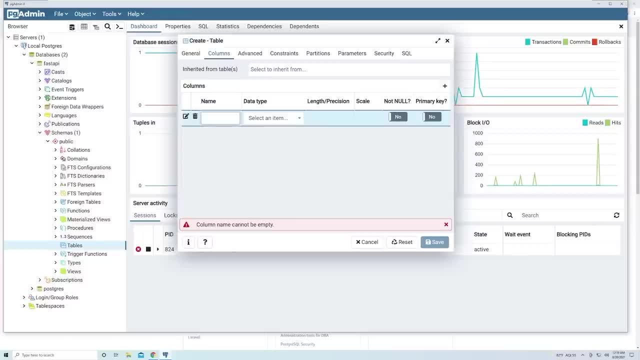 And you know a product is going to need a name, So let's give it a name, And so we'll call this column Name, because it represents the name of a product. Then we have to give it the data type. 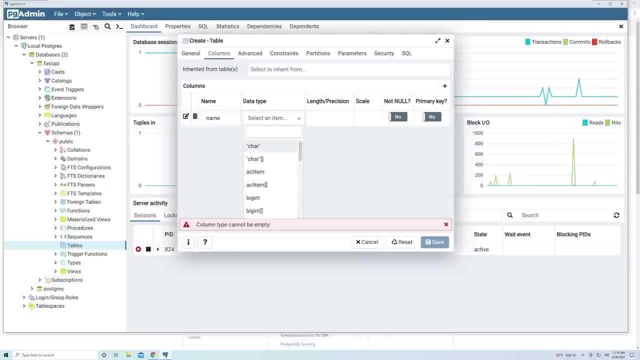 As I mentioned, there's going to be different data types that closely resemble or match the data types of a programming language. So a name is going to be, you know, a certain amount of text, right? So we need whatever data tape represents text. 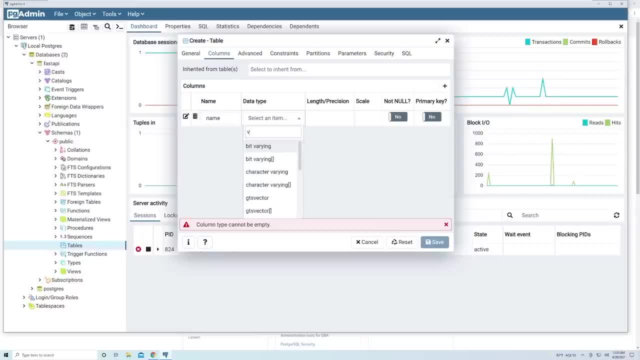 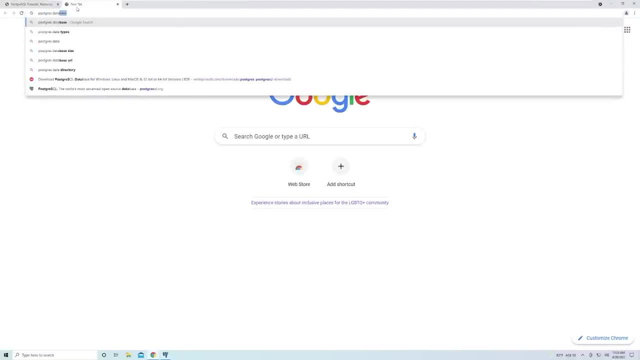 And so we've got a couple. We do have text, And then we also have a varying character or character varying. This is the one I'm going to ultimately use. So we're going to select character varying And if you actually want to see the difference between these, I recommend you go online search for Postgres data types. 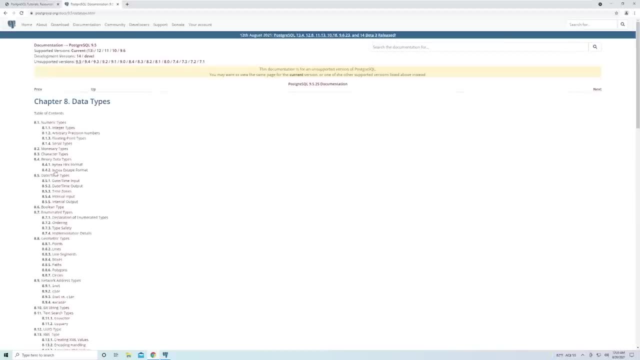 Right, And then just, it's usually chapter eight of the documentation. You can select this, And then this is going to give you a breakdown of the different data types And it's going to break it down based off of, you know, numeric types. 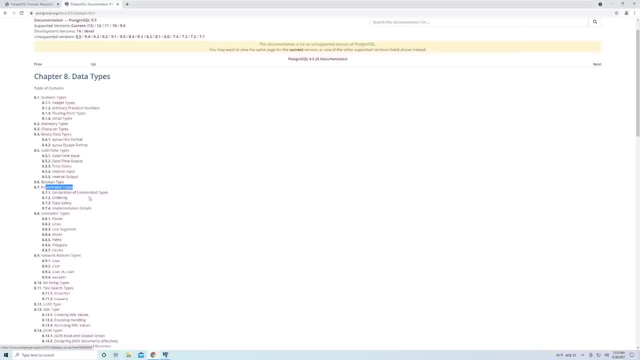 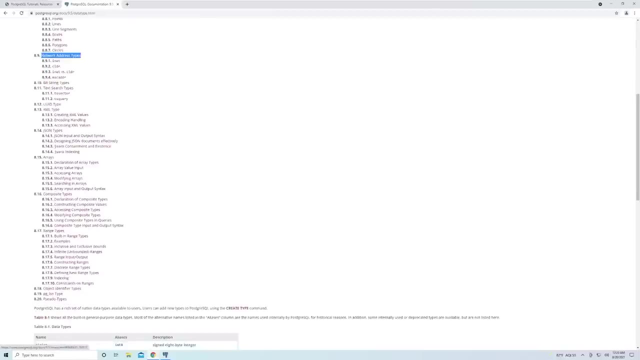 We've got a date time, a Booleans enumerated. We've got you know. if you want to represent IP addresses, we've got a data type for that. So there's a ton of different data types. I definitely take a quick read over all of these. 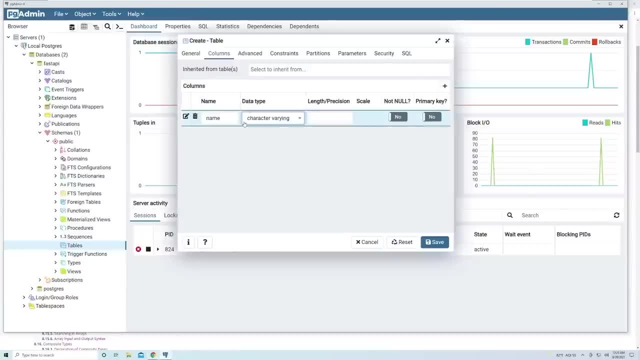 However, we're just going to stick to the basics. So if you don't want to go through all of that, then we'll stick to just the core fundamentals for now. So anytime we're working with text, we're going to use character varying. 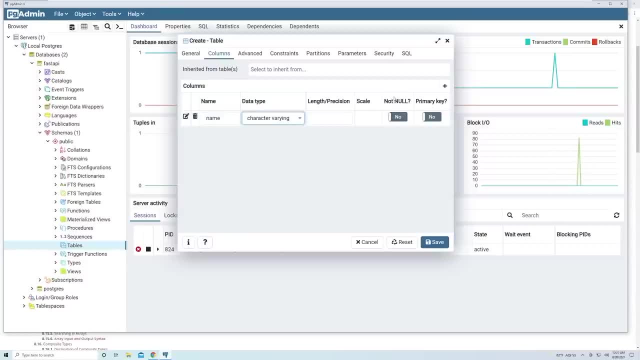 And then, as I mentioned, we've got a couple of options. So we've got the not null, And so right now it's set to no, which means that technically we can leave this entry blank, so we can create a brand new product with no name at all. 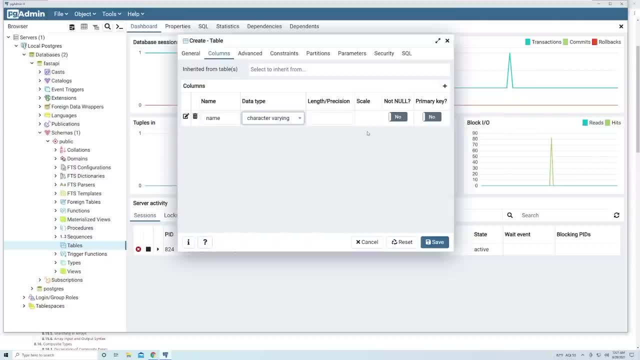 And then Postgres is going to put in a value of null if we do that. But if we think about our application, right, would we really want to be able to create a product without a name? Doesn't really make sense. So I think we should set this to be yes, so that it actually throws an error if we try to do that. 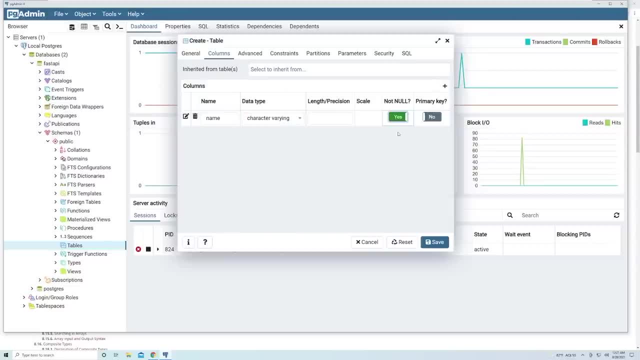 And you'll see a flag for a primary key. So we get to specify which a column is ultimately our primary key. I don't think the name of a product should be a good primary key. We need the primary key to be a column that really emphasizes what makes each entry unique. 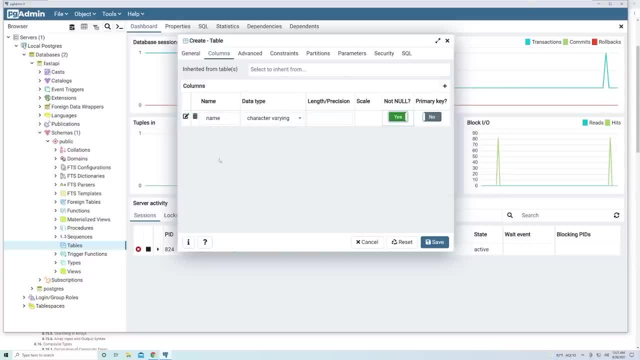 And I don't think the name name actually does that. So we're going to leave that set to no for now, And we're going to add in a new column, And this time we'll add in, let's say, the price. And so now we 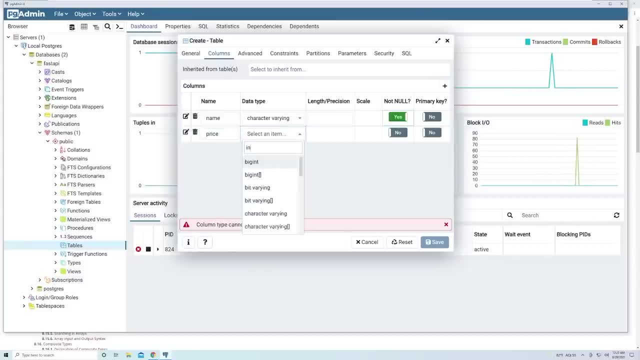 have to specify a data type. So for numeric data types we have an integer which is going to be whole numbers, which probably isn't a good data type for prices because we need decimals. We do have numeric And there's a couple of other ones. So if we go back to 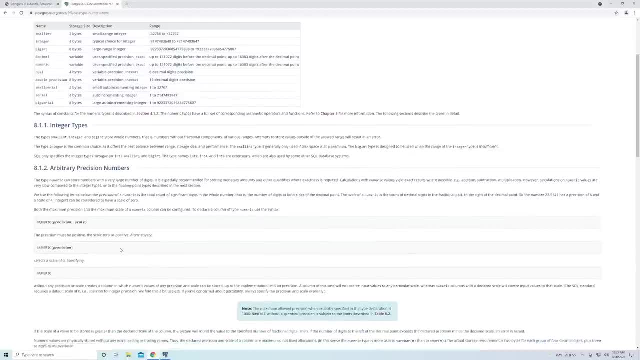 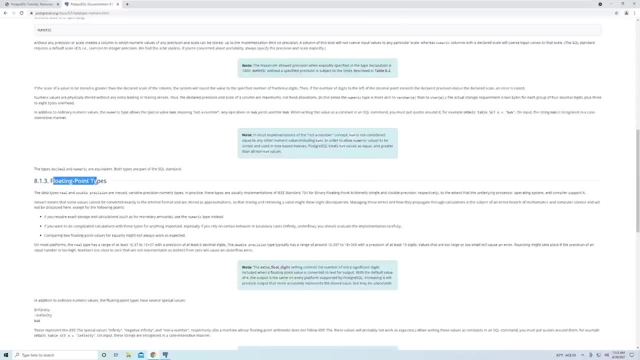 our documentation hit numeric types. We've got numeric, So this allows us to specify also decimals as well versus integers. And then we also have floating point types as well. Either one of these can be used. They operate a little bit differently, but both. 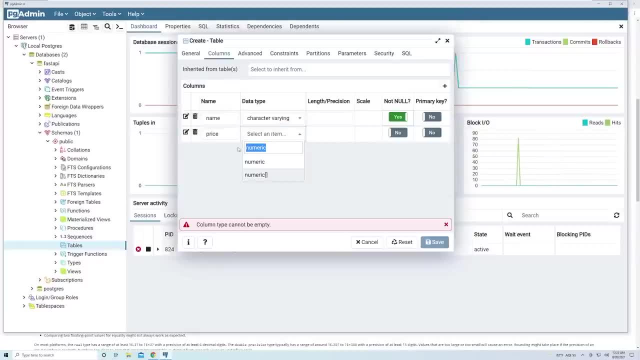 of them will work. But since I want to keep things simple and I don't want to confuse you guys too much, I'm just going to use an integer to define a price. And I know technically there's no application that would ever use an integer to represent price, but I want. 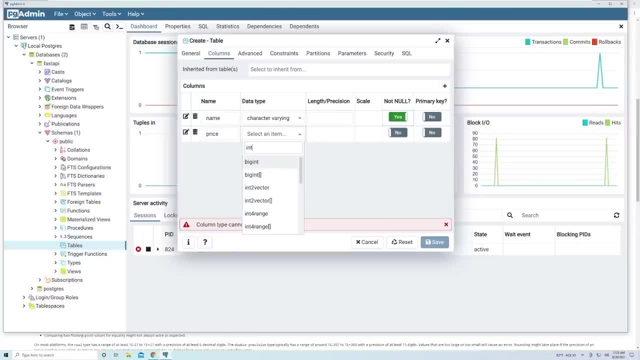 to keep this simple And I actually want to show you guys something unique. So you see that there's a couple of different types of integers. We have, first of all, a plain old integer, We've got a small int, And then we've got a big int. So what is the difference between all of those? Well, 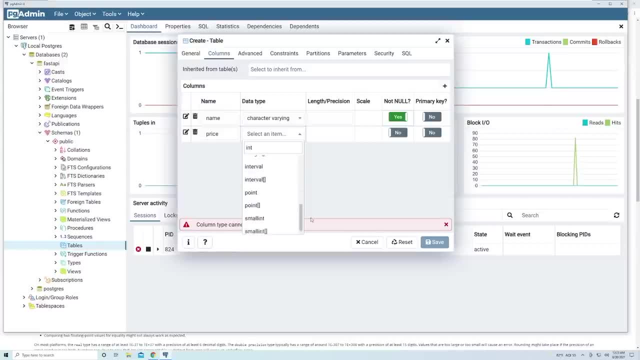 it's the number of bits that we have. So a small int has the fewest number of bits, which means that the maximum number we can go to is going to be a lot smaller versus a traditional integer, And then, if we need to go up to a really high value, we're going to use big. 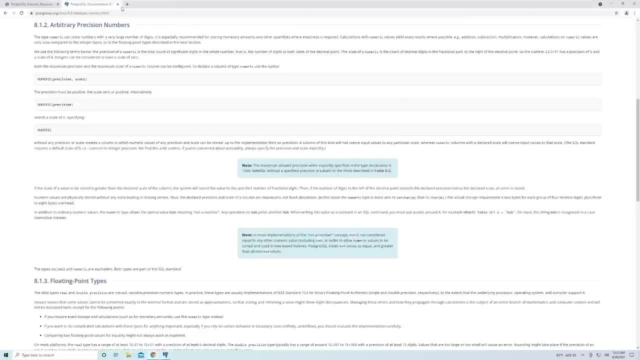 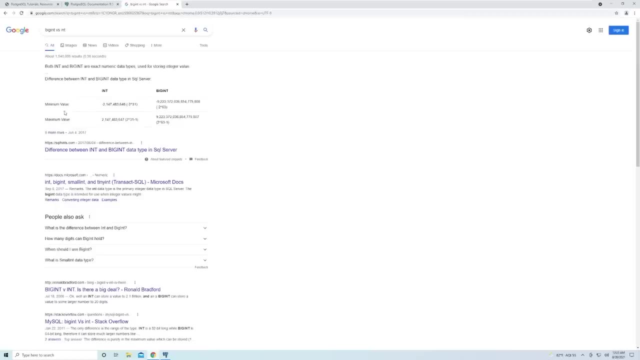 int, Which is going to have the most number of bits. And if you want a good explanation, just search for what is the difference between big int versus int, And so we can see here the difference between them is: you can see the minimum value and you can see the maximum. 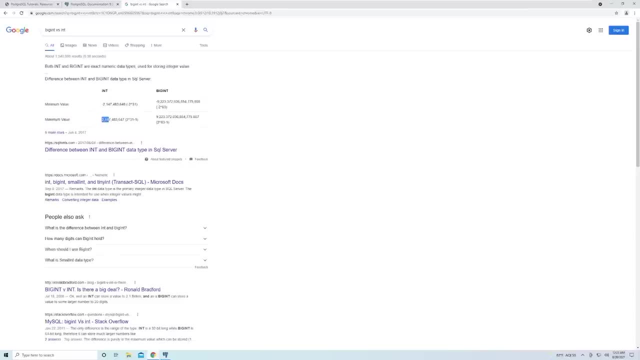 value And so I think that's what minus 2 billion to 2 billion, So we get it in the negative and the positive direction, versus a big int which is negative, 9 to 9 billion. So you got to figure out what's the best fit for you. If you don't think, you'll even hit. 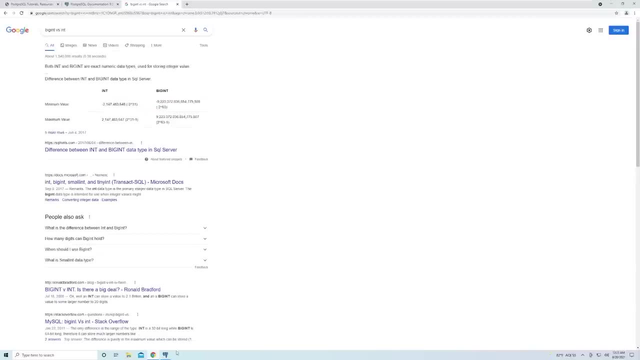 2 billion, then there's no reason to go. So I'm just going to leave this as a plain integer. We could definitely get away with the small integer, but let's not worry about that. I don't think we're ever going to have. 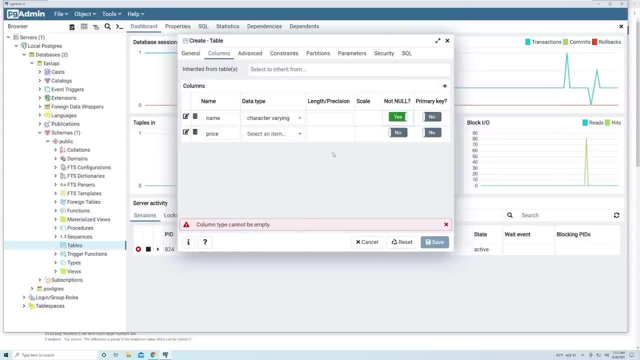 a product that's going to be 2 billion dollars, but that's fine, All right. And then, once again, we have the not null option. So it doesn't make sense to create a product that doesn't have a price, So let's make sure that's not nullable. 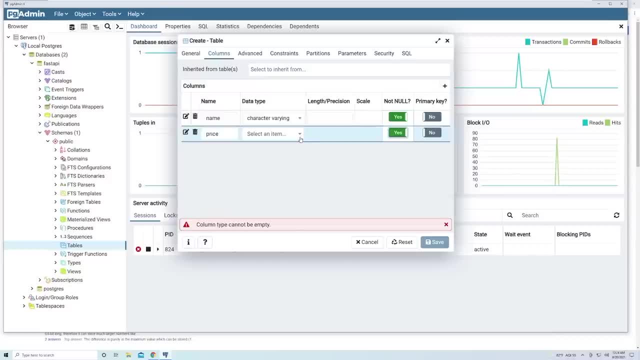 And then the length and the precision. this is for floating points, So you can say, like: how many decimals do you want to support For an integer? though it shouldn't matter, And it looks like I didn't properly select this. We'll do integer, All right. And then the last thing that we need is each product should have: 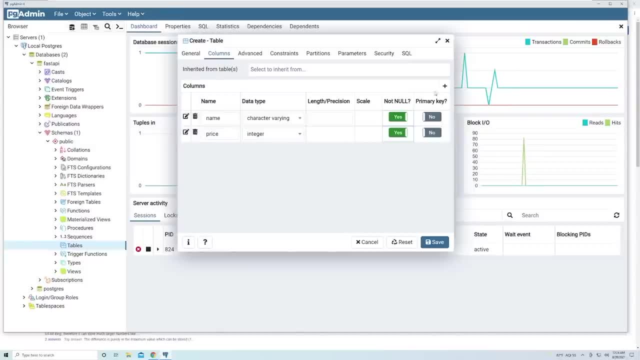 a unique ID right And, like I said, a lot of our tables are going to have an ID column. So here we're going to create a column called ID, And so what kind of data type should we use for this? Well, I think what makes sense is an integer right. An ID is just going to be some random. 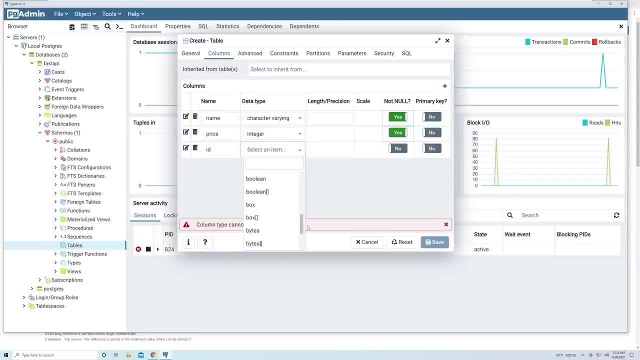 number. So we could use int- big int, or something like that, And then we're going to have a unique small int, And so let's just say we'll use an integer. I'm going to search for integer. However, I don't actually want to leave it like this. I did mention in one of the previous 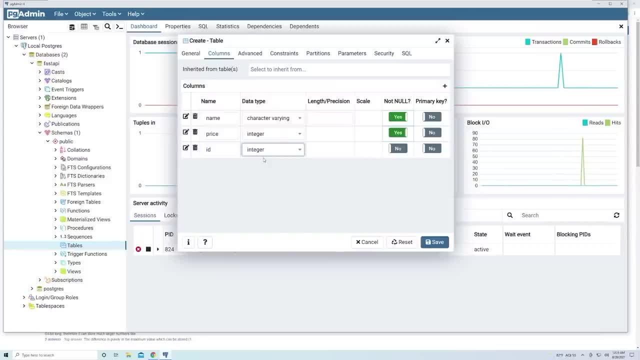 lectures that most databases support the ability to automatically generate a ID for you, So I don't want to have to be the one responsible for creating an ID and then putting that information into Postgres. I want to just provide the name and the price And I want Postgres to generate a unique. 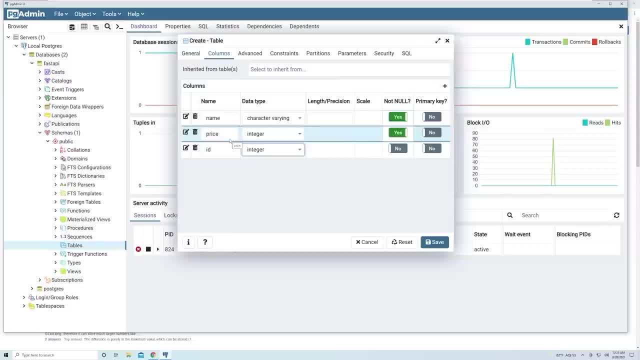 and random ID for the product. So I'm going to go ahead and create an ID for the product And I'm going to go ahead and create an ID for that product. So how do we do that? Well, it's pretty easy. There's a data type called serial, And so a serial is just a regular integer. However, it 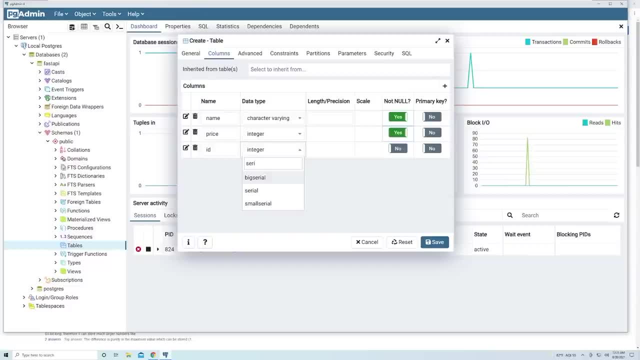 automatically creates a random number, And it's actually not a random number. What it does is the first product we create will get a value of one, The second one will get a value of two, And it'll just increment by one for each product we add. So it's going to ensure that every single product we 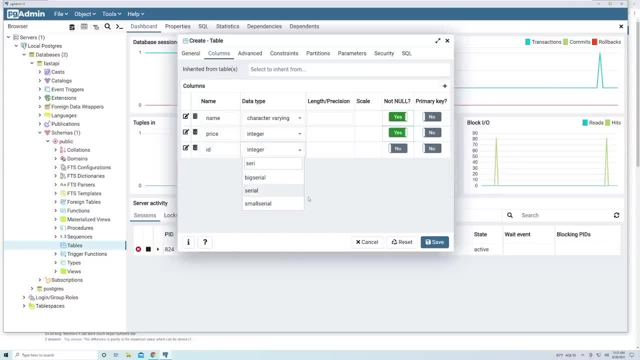 create gets a unique ID, And so that's what we're going to do. So let's go ahead and create a integer value for the ID column And, like I said, we do have small ints, big ints and regular integers. This is the same thing, but it's just auto-incrementing for those three kinds. So I'm 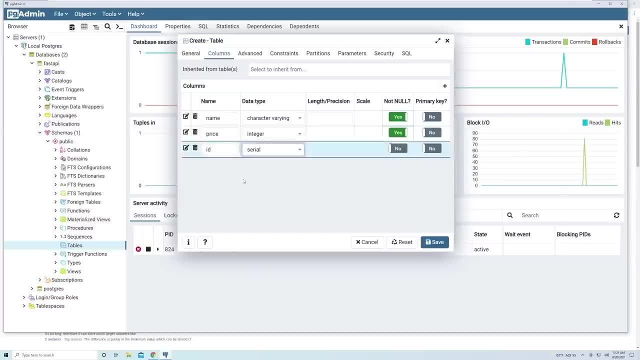 just going to say it's going to be a regular integer that increments by one automatically, And then this is going to be what's going to be the primary key. We know that the ID has to be unique. I think that makes sense to make it the primary key, And I think, for now, this is a good. 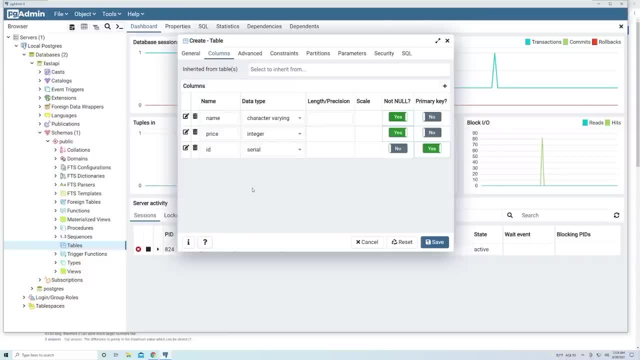 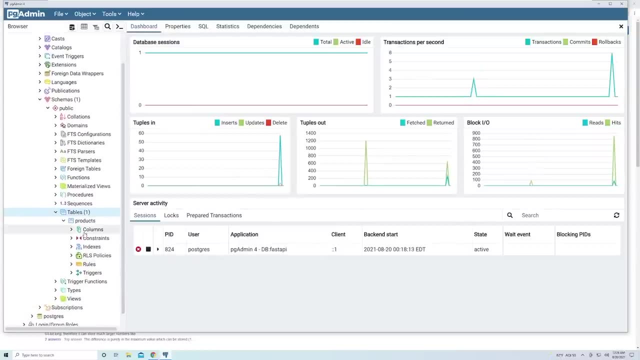 enough starting point to learn about SQL. So let's save this. And we have then successfully created our first table, And so under tables you'll now see our products table. So let's start playing with this products table. Let's create entries, Let's delete entries, Let's really start to have fun with it. So right-click on it. 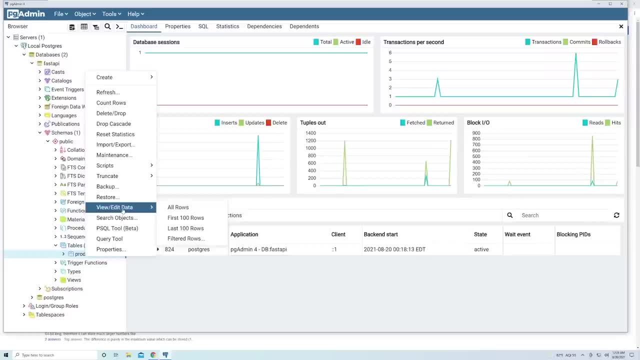 and select view, edit data And then you really select any one of these. If you select all rows, what it's going to do is it's going to fetch every single entry that we have in the database and show it to you. We don't have anything in the database, so it doesn't really matter. So let's go ahead and 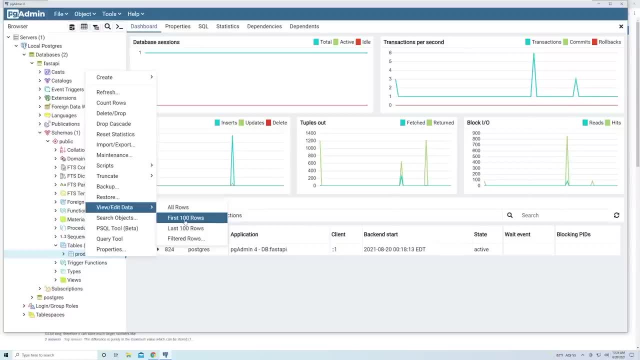 do that. If you select first 100 rows, it's going to grab the first 100 rows in the database, And if you select last 100 rows, it's going to grab the last 100.. Now, if this was a production server or? 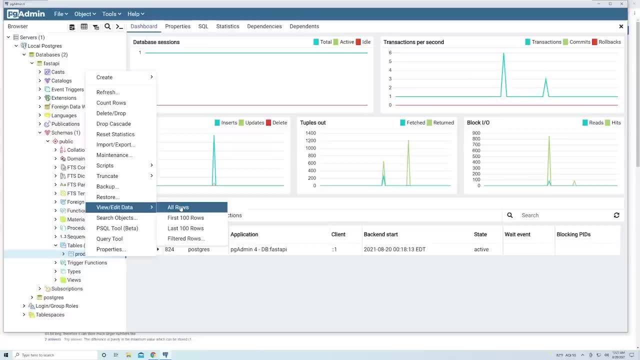 something like that. we might have millions of entries, So you may not want to do all rows and then just get flooded with all of this data. So you may want to select one of these or filter out the rows based off of some criteria, But we have no actual data on it, So I'm just going to select. 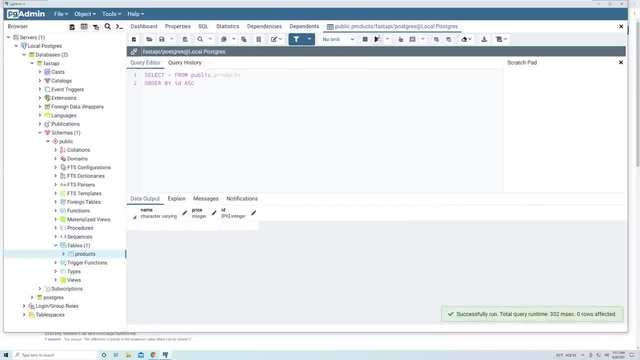 all rows And you'll see that within pgAdmin we have these different tabs. So it opened up a new tab And you see that there's like a little pop-up window. So if you can pause it and rewind, it says that it actually ran a query. And so what it did is it ran a query to retrieve all the rows because 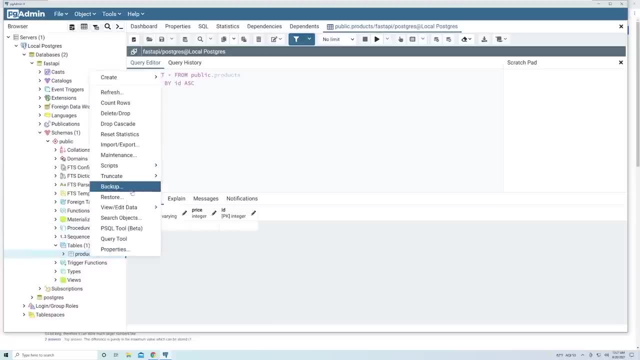 that's what I selected. right, I selected, you know, get me all of the rows by selecting all rows. And if you look at this query editor right here, this is the actual underlying SQL that it ran. So it ran: select star from my products. table order by ID in an ascending fashion. So it's going. 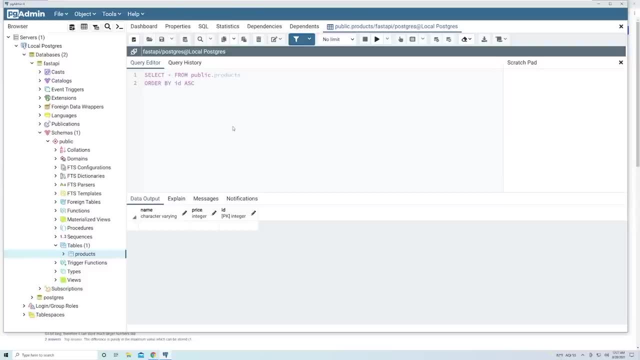 to take the product with the lowest ID number and the next product with the second lowest ID number, and it's going to keep incrementing up. We've got nothing in our database, so it didn't return anything, But I think it's cool that it does show us the underlying SQL. Now, like I said, we don't. 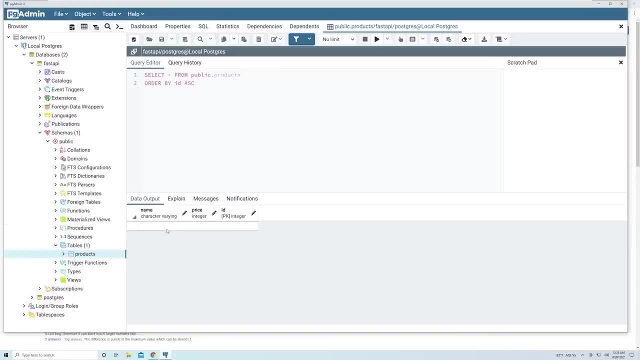 have anything in our database at the moment. So let's go ahead and create our first entry. So I'm going to create select, this column, and I'm just going to give it a name. So this is going to be a, let's say, a TV, And let's give it a price. I'll say this is $200.. 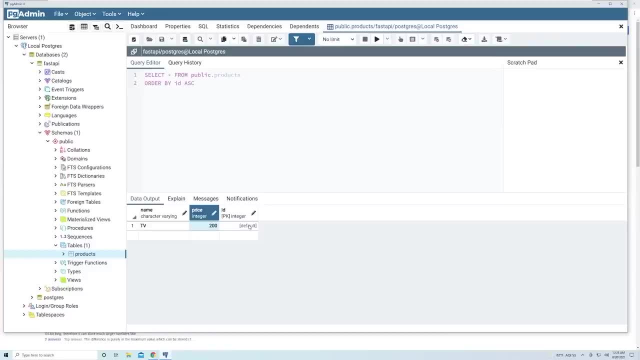 And then the ID. this is going to be automatically generated, so we don't need to provide a value. And so at this point you may be thinking: well, it looks like we created an entry right. We have our TV price of 200.. Well, not exactly To actually store this data in the database. Right now we're 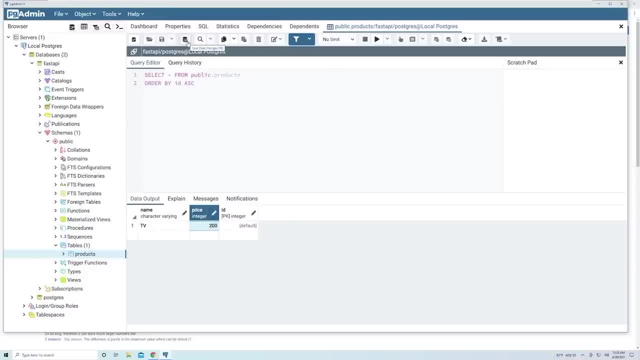 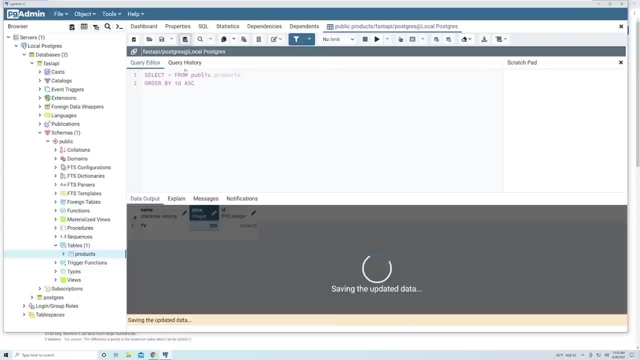 just proposing changes. we have to select this button right here. So if you hover over this, this says save data changes. So when you select this, this is actually going to push this data into the database. So let's do that. You can see that the data was saved successfully And now it's. 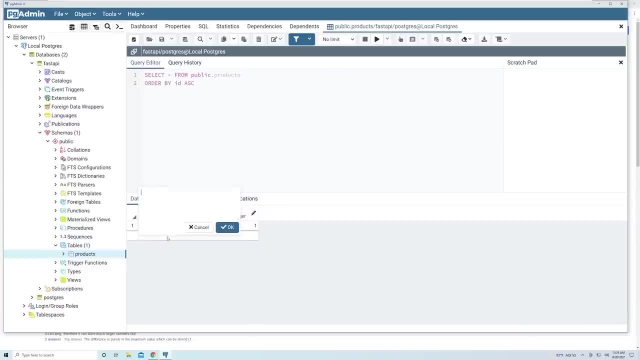 actually in here in the database. So let's create a new entry. I'll say: this is a DVD player. I don't know if anyone uses these anymore. And then let's give this a price. I'll say this is $80.. And then 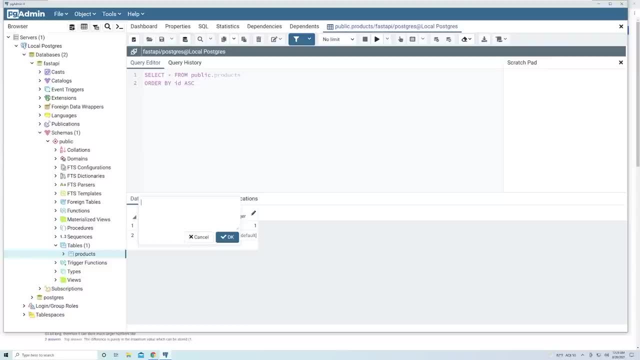 we can. we can just keep adding as many as we want. So let's add in a remote- This is going to be 10 bucks And you'll see that anything that's kind of bolded, so you notice how TV isn't as bold as 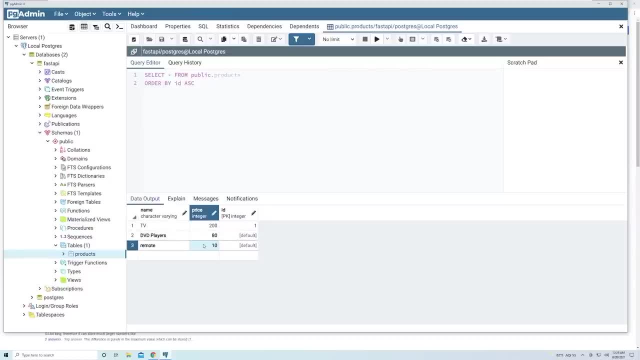 DVD and remote. So bolded means we haven't actually pushed it out to the database, It's just proposed changes So we can push out both of these at the same time by pressing this again. So we push that and then you can see that they got pushed out. and take a look at the ID column. 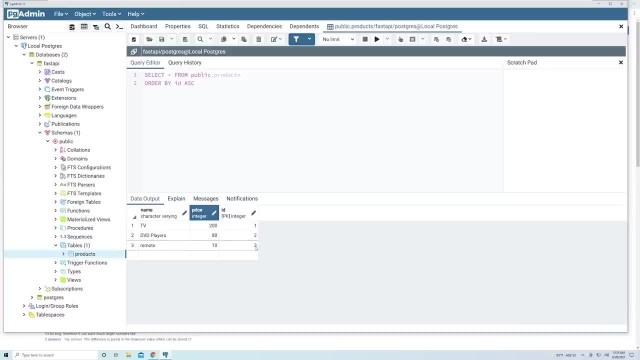 right, The first item got an ID of one, the second one got an ID of two and then three, and it just keeps. it's just going to keep incrementing. Now let's have a little fun. Let's create a new item. This time let's create, let's make it a microphone or something. 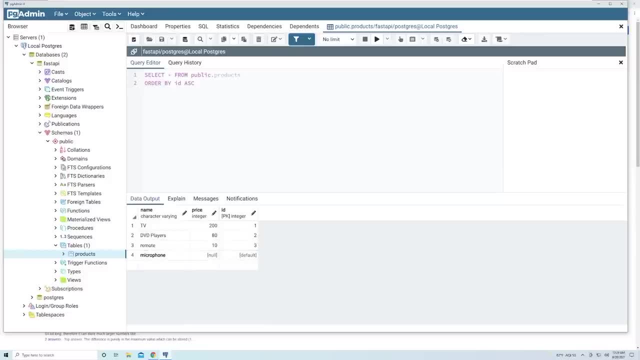 And let's leave this price column blank And let's see what happens. So now, if I press this, take a look at this error: null value in column price. So we left this value empty, So Postgres interpret as null. but we set the column to be not null, So we told posters to do a check. 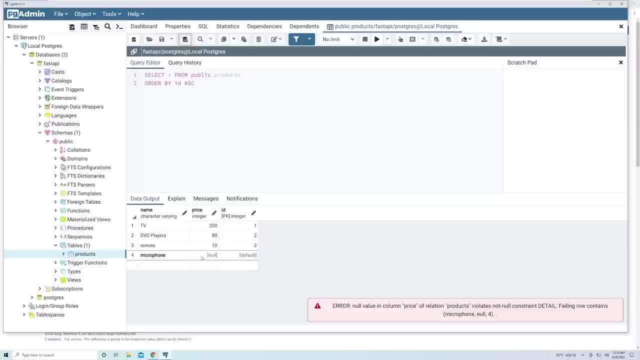 and say: Hey, listen, if we ever don't provide a value, we want you to throw an error. So this is forcing us to provide a value for this, because creating a product without a price just doesn't seem to make sense. So let's give this a price, Save that, And so now that works. 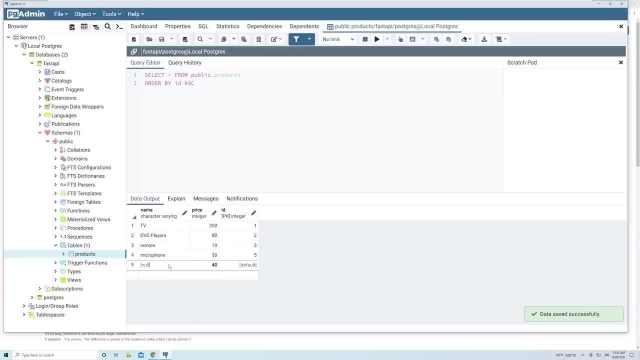 and then this time, let's try creating a product with a price, But no name. this time, Right? So what do you expect to happen? Well, since we set the column to be not null, it's going to throw an error, or it should, hopefully. And look at that null value in column name. So once again, it's. 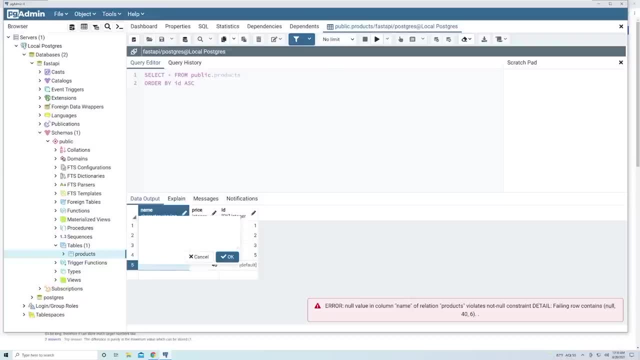 not going to be supported. It's gonna throw an error. So let's just give it a name. Let's say: this is a car, the world's cheapest car, hit. okay, save that That's been successfully added. All right. so now that we've kind of played around with it a little bit, let's make this a 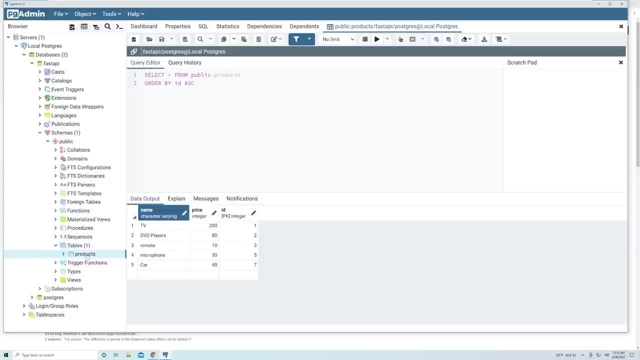 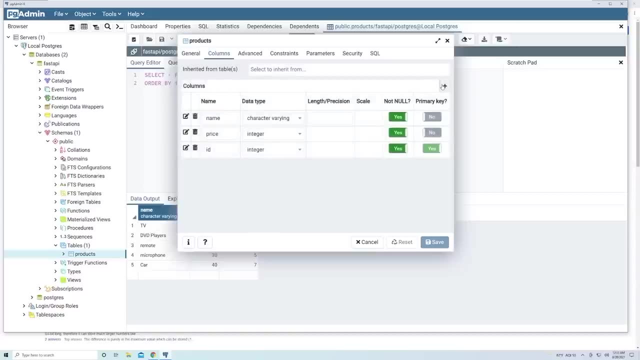 little bit more interesting And let's add in a brand new column to our products table. So right click on the products table right here and select properties, And under columns we're going to add in a brand new column. So we're just going to follow the same steps And this column is going. 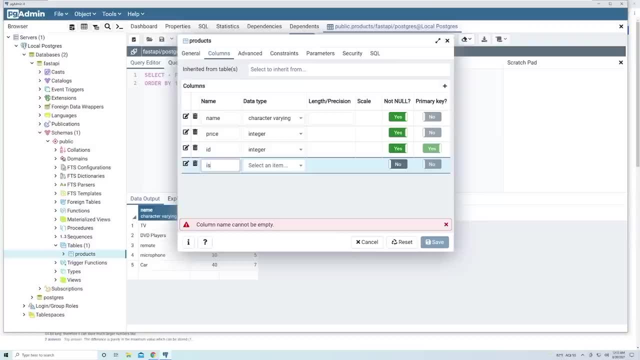 to represent if an item is on sale. So I'm going to call this is underscore bull. Sorry, not is the underscore bull. it's going to be is underscore sale, And it's going to be a simple Boolean as a data type, because the idea is going to be set to true, which is going to be set to true. So 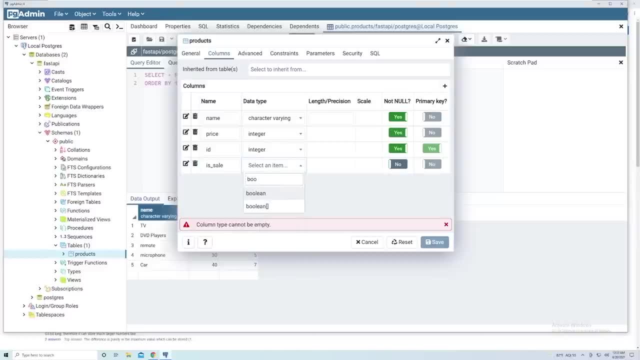 we're going to set it to true, which means the items on sale, or false, that the item is not on sale. So we'll do Boolean And then everything else we're just going to leave deep by default. So for not null, we're going to leave this to be no. So we are going to allow the user to input a. 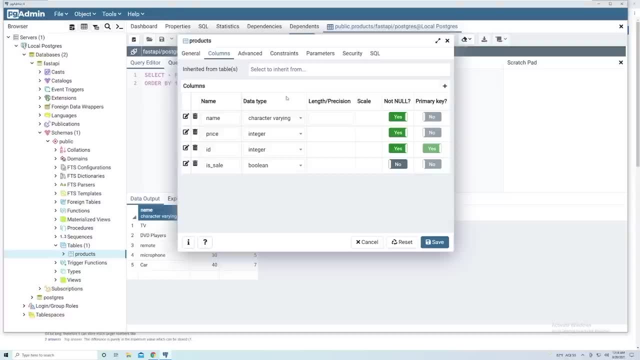 value of null. in this case, However, what we're going to do is we're going to add in an extra constraint, I guess Actually we're not gonna. we're going to set a default value. So, if the user does not provide, 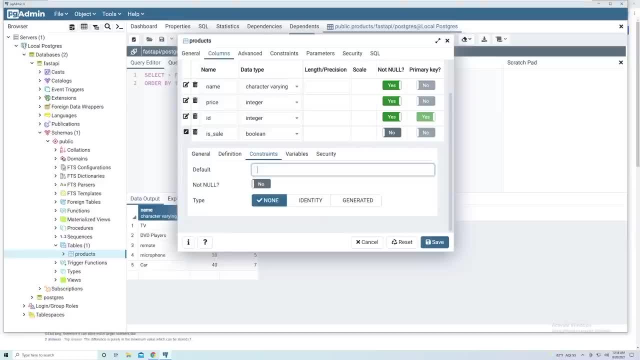 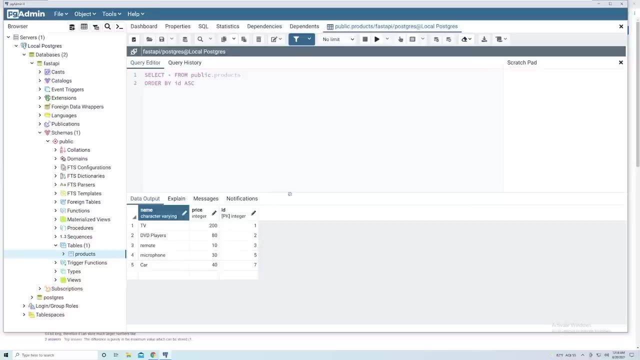 a property for is underscore sale, we're going to give it a default value and say that by default, if a product doesn't receive a property for sale, it's going to be set to false, So it's not going to be on sale. So let's hit save, All right, and then right now you don't see a new column, But 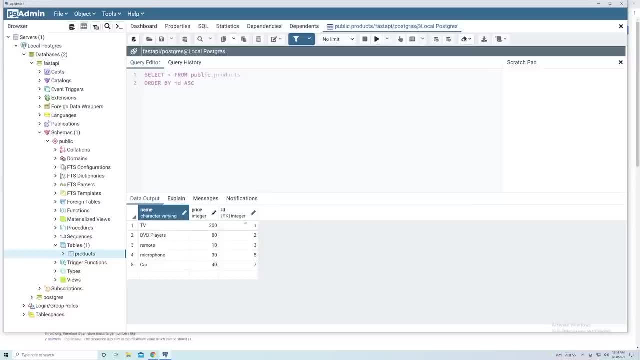 that's because you don't see the new is on sale column, But that's just because we need to refresh this page, So let's go under object. I think we could do it here. I think it should be a refresh And this should provide me. the value is set And I think if we cool it now, it's going to show up. 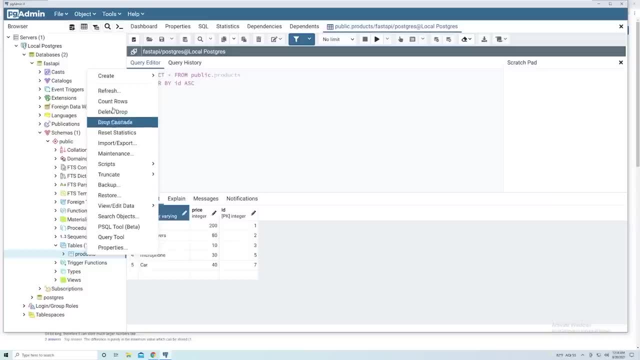 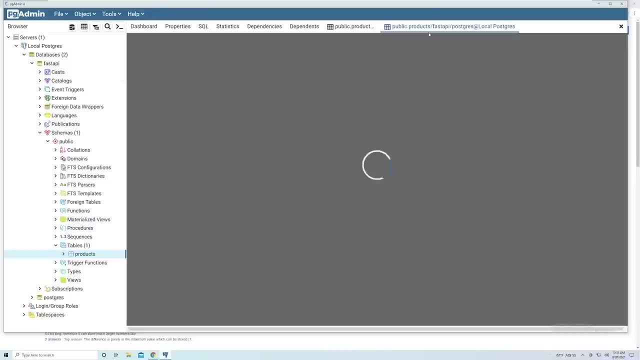 BOA plugin with aosition here At the very top that we saw it here. I didn't do anything, So I think we're just gonna do the same thing as we did before. There should be a way to refresh this, But it looks like if I just press it here it doesn't do anything. So instead, 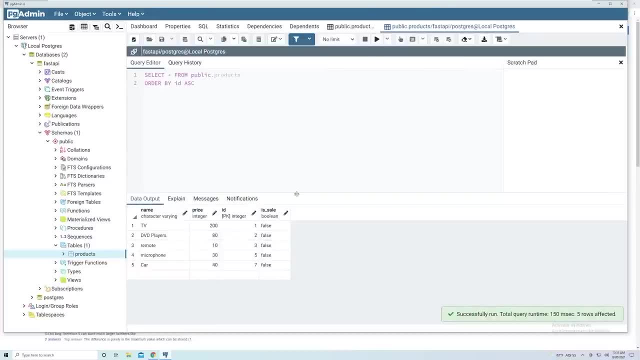 I'm just going to do a view: edit data all rows again. it's going to open up a brand new tab And now we can see the is underscore: sale a column here. And what's awesome about this is that because I provided a default value, 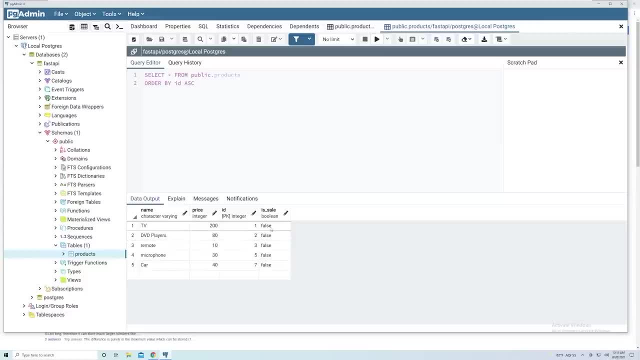 it went to all of the other items in my database that didn't, that were created before this column was created, And it provided the value of false because I said, Listen, if, if the value is null or if we didn't provide that data, go ahead and put in the default value of false. And so now, 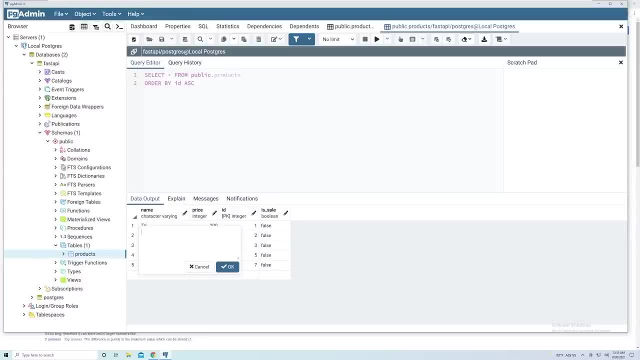 if I create a brand new item and I'll say: this is for a pencil, And the pencil is probably only $2. Now, since this can be set to null, I'm going to just leave that blank. And now, if I save this, 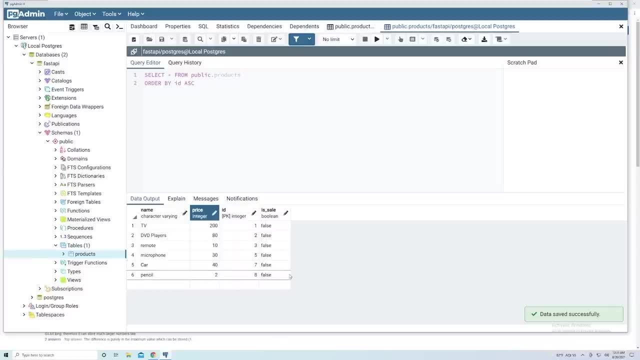 take a look at this: it gets the default value that we provided. So you'll see that for a lot of your columns you're going to want to provide default values if you expect it to be frequently inputted without a value and you want it to receive a default value. And now, once again, 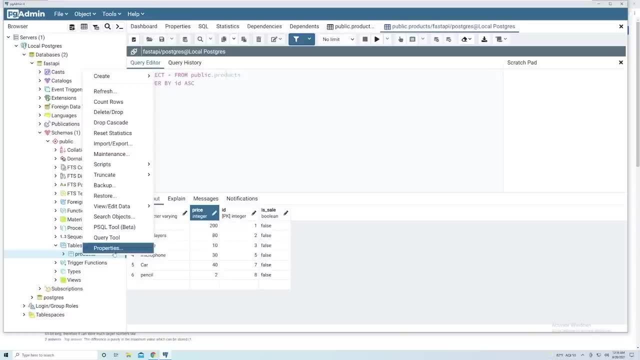 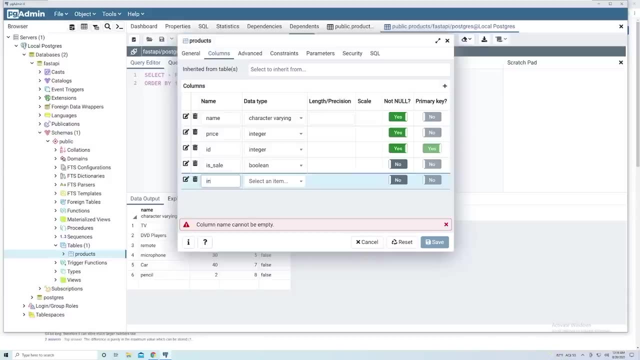 I'm going to actually create a brand new column once more, And then we'll go to properties, we'll go to columns And then we'll add a column And we'll call this column inventory. So this is how many of the items that we have in stock, And so here this is going to be an integer. 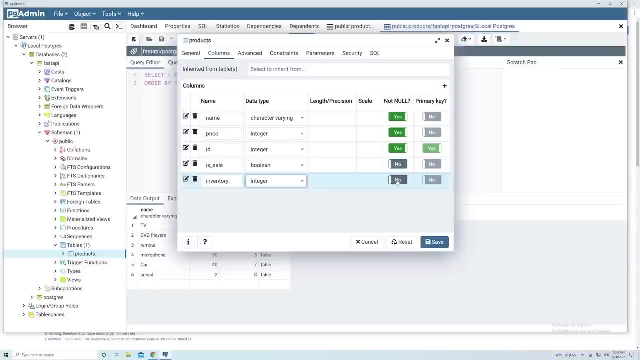 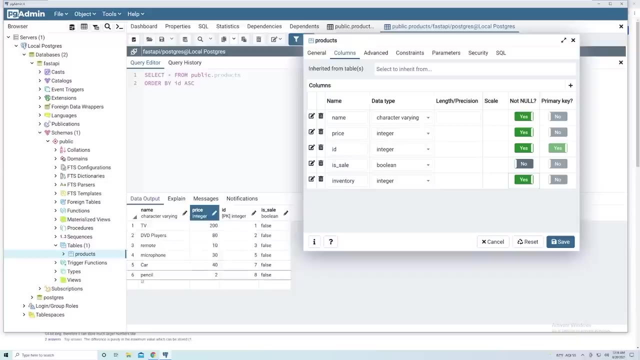 And I think it makes sense for, in our application, to have a value for our inventory, we shouldn't leave it null. So I'm gonna set it to yes, And I want you guys to see what happens when we hit save, Because the big issue is right: this column doesn't exist at the moment And so all of these items were. 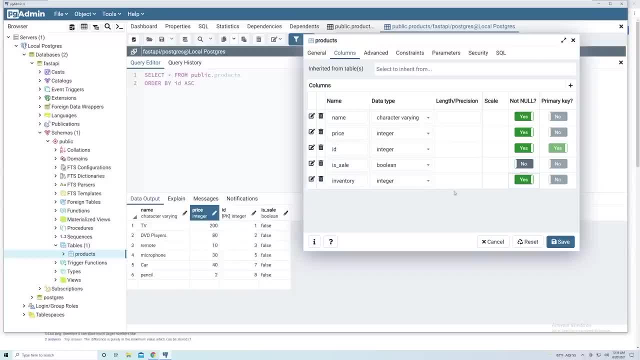 created. before there was an inventory column that was created. However, this column has a not null value, but it doesn't have a default value. We gave is sale a default value. So Postgres was smart enough to go into all of these pre existing items and give it a value of false. Well, what's? 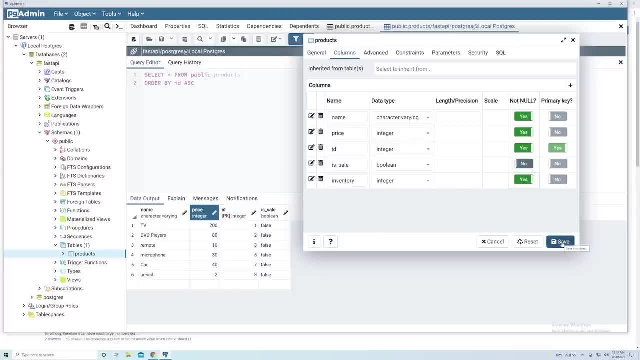 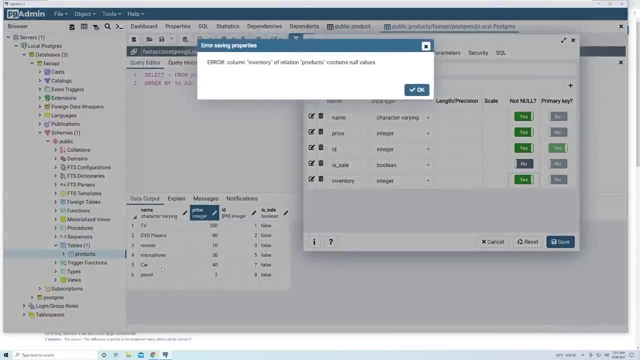 going to happen with the inventory. I didn't give it a default value, So let's see what happens. If I hit save, it throws an error. it says column inventory of relation products contains null value. So it's basically saying all of these products that you had before don't have a value. 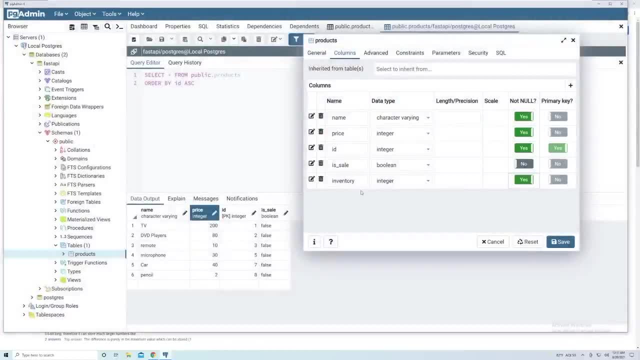 for inventory. So at this point you know you have a couple of different options. You could delete your all of the previous products if you wanted to, But since this is a development environment, that's not a big deal If you're in a production. 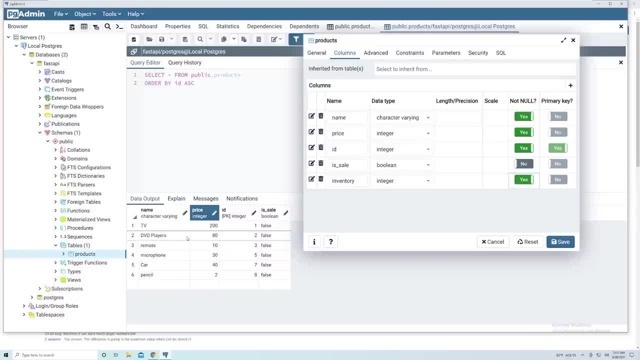 environment. that could lead to issues. Obviously, you don't want to delete your production data, So we could just give it a default value, like we did before, And so I can just go back into what's out there. we want to select this little button, go into constraints. 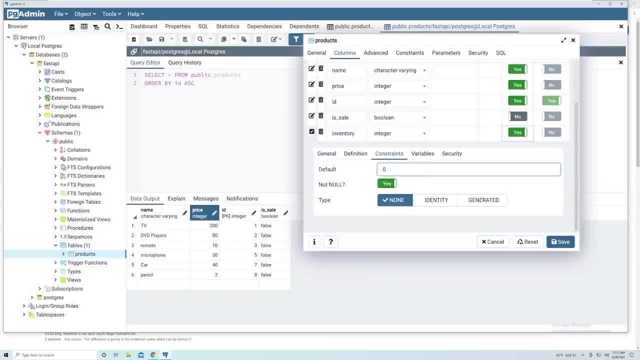 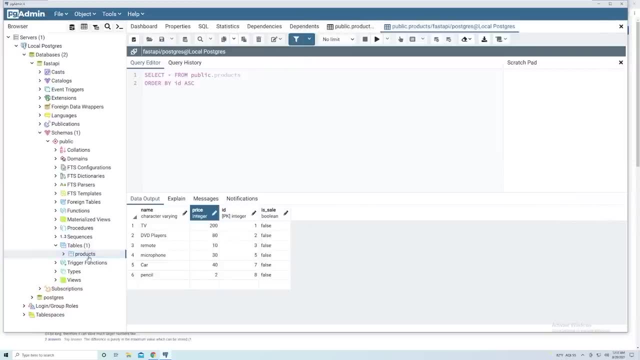 and we'll say the default value isnesses. there's going to be zero items. let's hit save. And once again, I'm just going to open this up- Lyric B Polish noticed that her mind was clear when she was floor. If you're not sure what Sheer Is, 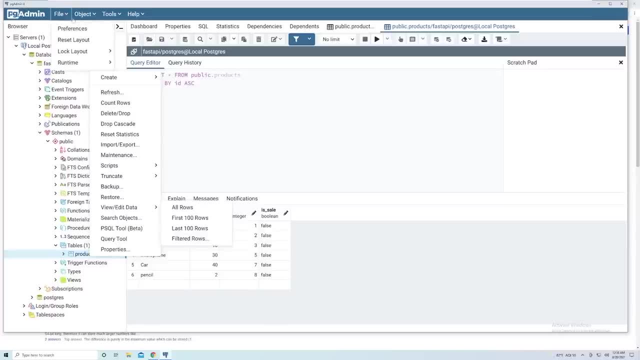 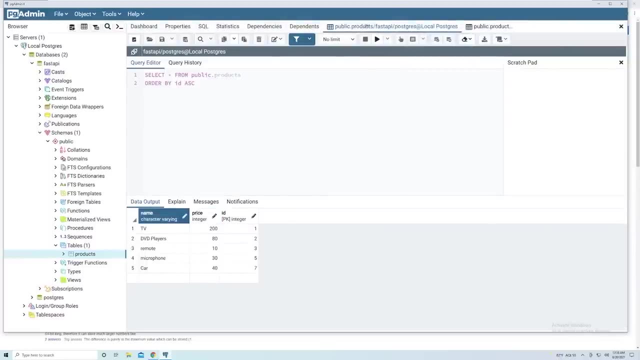 to refresh it. I know there has to be a way. I can't find it, So it's okay, we could just open up this again And then we can just delete these. I don't want too many of these, I don't. 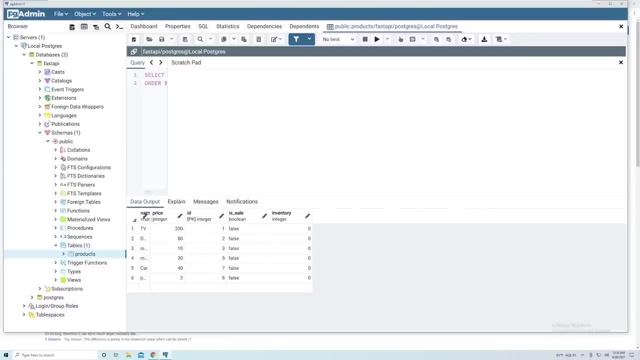 know why it's got squished up like that, But because we provided a default value, it all. it got all values of zero. And so now if I create a brand new item and I'll call this one, this will be a pencil sharpener. We'll give a price of $4 is sale, I'll set to be. 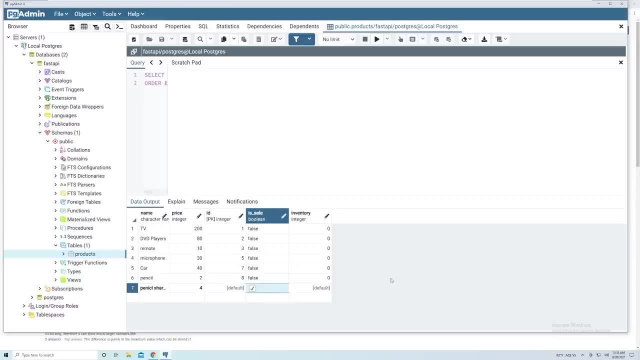 true, True. And then, if we don't provide an inventory, it's gonna get that default value of zero. Alright, so I think we've almost wrapped up our schema for our products table. However, I want to add one more thing, And this is something that's pretty common. 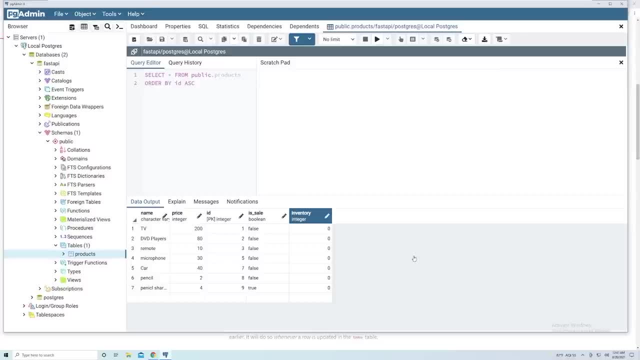 Anytime you create an entry within almost any other table, you usually want some sort of timestamp, right? So what? when did we add this product? When did this user create as account? When did this user create this post? right? So anything that we add into. 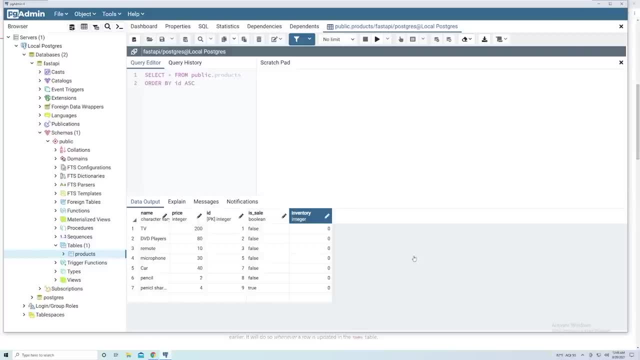 our database or an application, it is generally best practice to store when that item was created, because you never know when you need to know that information. So let's create another column And let's see how we can work with timestamps. So I'm going to right click. 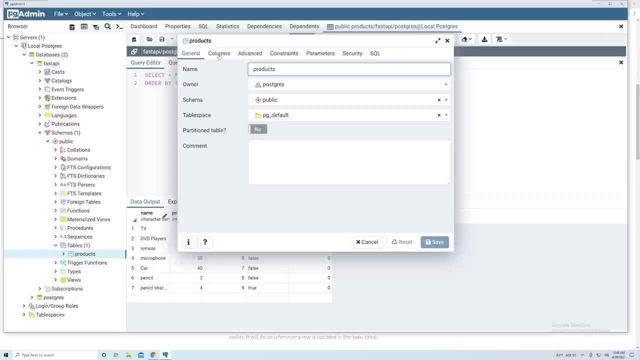 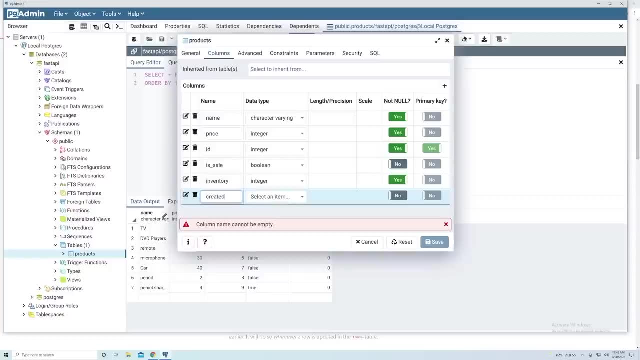 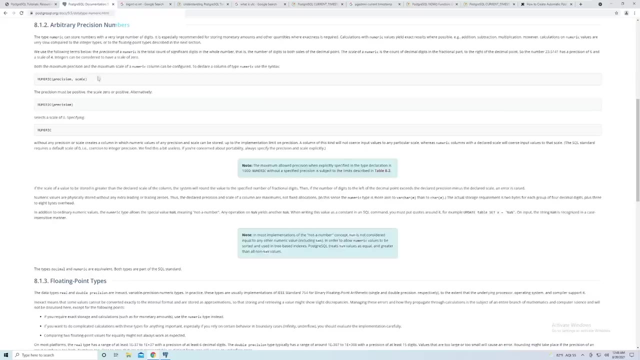 on products, as usual, go to properties And then, under columns, we're going to add in a new column And we'll call this column created that, and then here we have to select something that represents time. So what I recommend you guys do is just go to the documentation And then look at DateTime types. So there's. 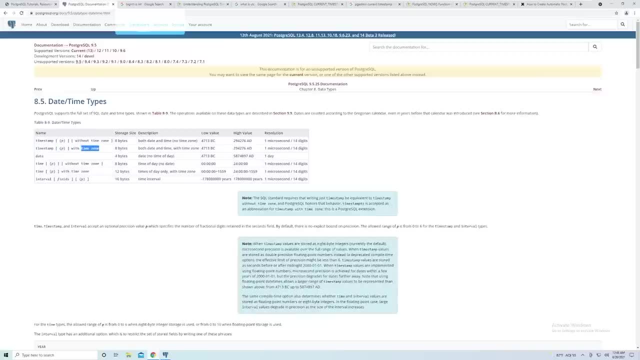 a couple of different ones, But what we're going to do is timestamp with timezone. So we got timestamp without timezone and then timestamp with timezone. We've got just the date, but I want the date time in the timezone, So that's the most detailed. So I'm just gonna 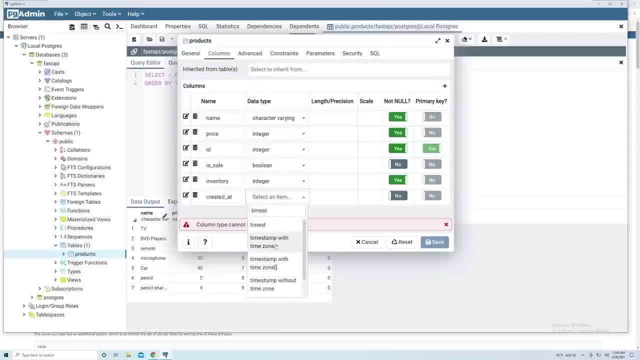 search for timestamp And we want timestamp with timezone And we obviously want this field always filled in. However, I don't want to have fast API API be responsible for creating the timestamp. I want Postgres to automatically create the timestamp for when the entry was created. So 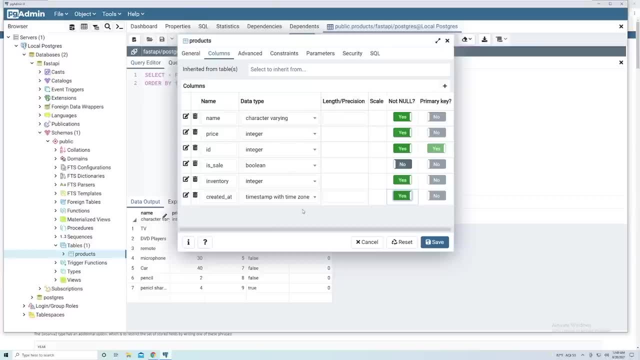 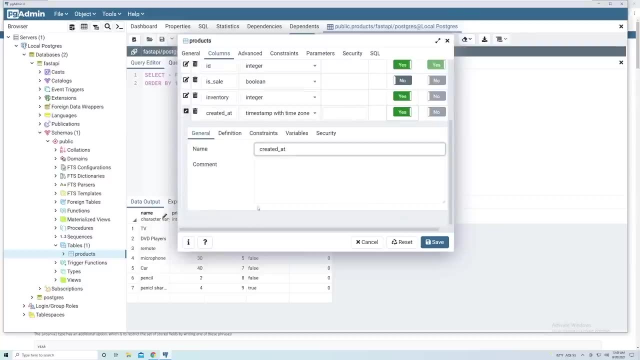 I want to be able to just create a product And then, as soon as it gets added to our database, Postgres will just fill it in with whatever that current time is. So how do we do that? Well, we can go into this right here. So let's configure this, add a constraint, And then here all we have. 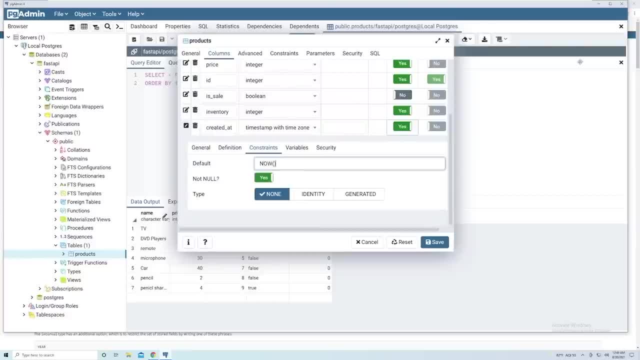 to do is for the default value. I want you to just write now: So what this is going to do is the default value for any product that gets added. it's going to run this specific command on the CLI, So this command just grabs what is the current time? pretty simple right now. 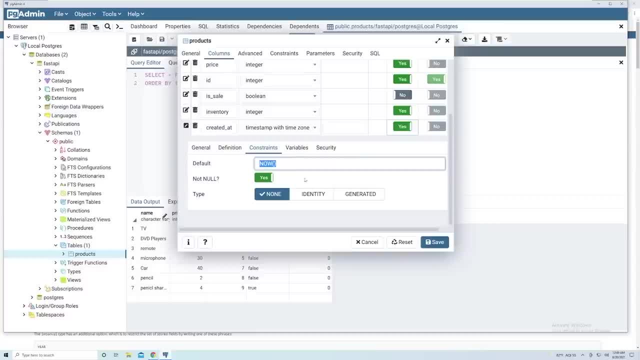 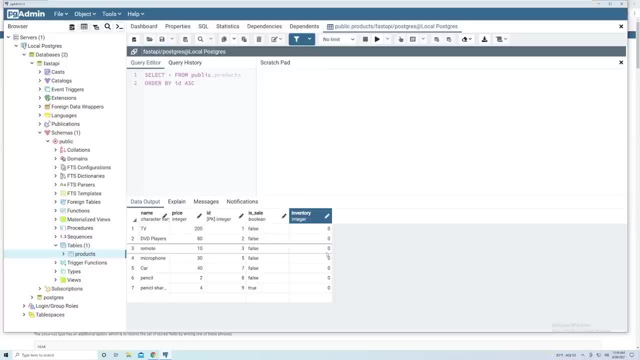 it. I think it's pretty straightforward: What time is it now? right? And so this will set the default value. So if I hit save at this point, since we had all of these other items that were created previously before there's a timestamp- 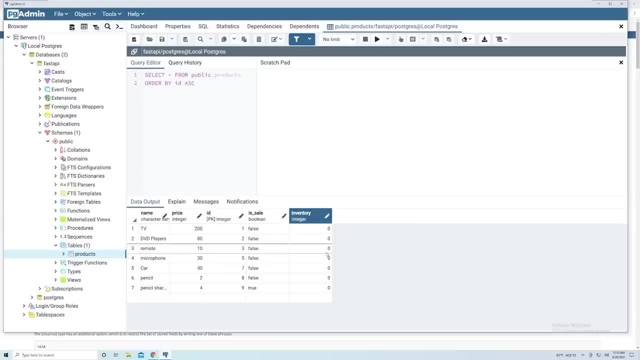 what it's going to do is it's going to set the created time to whatever time it is now, which technically that's not accurate because that's not when they were added, but these were created before we were smart enough to actually have a timestamp. 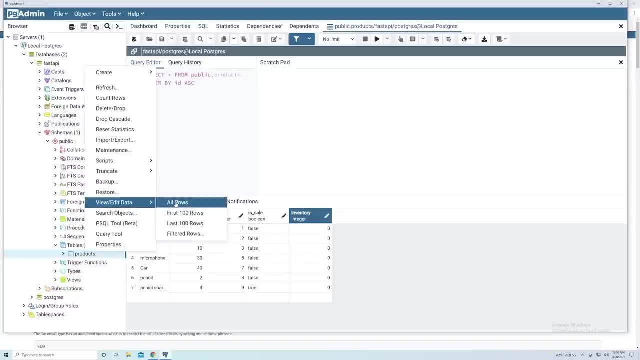 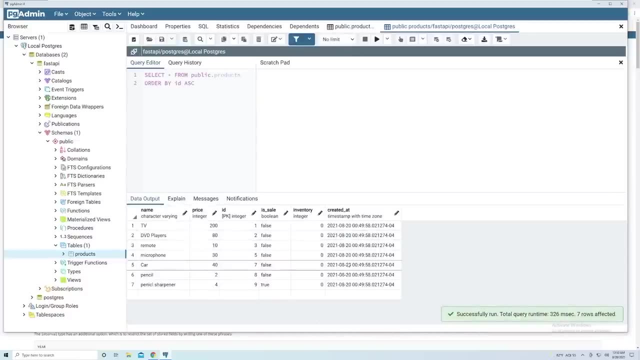 So if we refresh this- so I'm just going to do a view- edit all rows again. All right, you can see that they've all been given the same timestamp of whatever that current time was, And now, if we add in a new item, 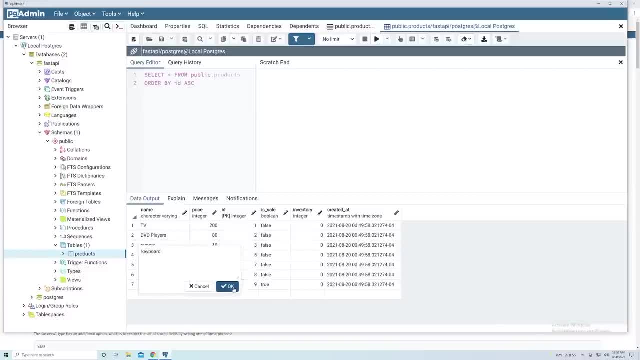 and I'll add in: how about a keyboard? We'll give this a price of 28.. Is sale? we can just leave that empty. How many in our inventory? We'll give it a 50 and then we'll leave this blank. 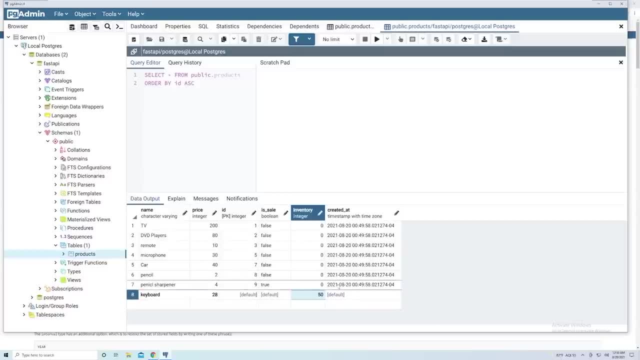 And so let's see if it automatically fills in what is the current time, And it should be later than this time, obviously. So hit save. And so if we just double check- yep, we got it- We could see that this is about a minute later. 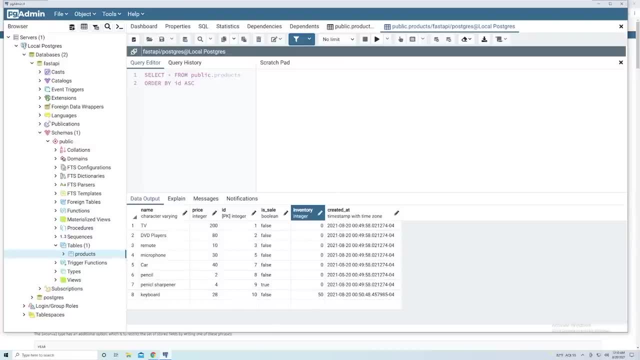 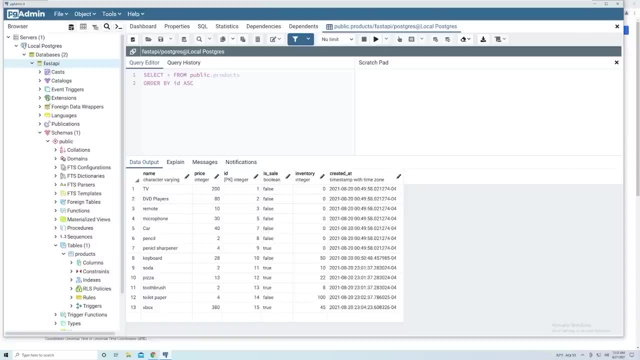 And so now we've successfully added the created at timestamp In this lesson, we'll run our first SQL command. However, before we do that, what I want you guys to do is create a few more entries within your database, And so you could see that off camera. 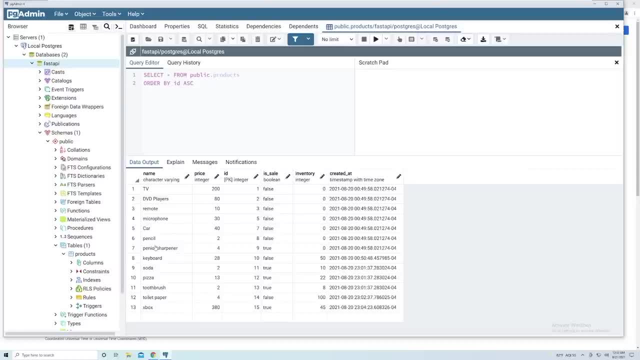 I added about six or seven more entries And you want to make sure that you provide enough varying data to your database. So make sure the price is all different, Make sure that the is sale Boolean is, you know, a good mix of true or false. 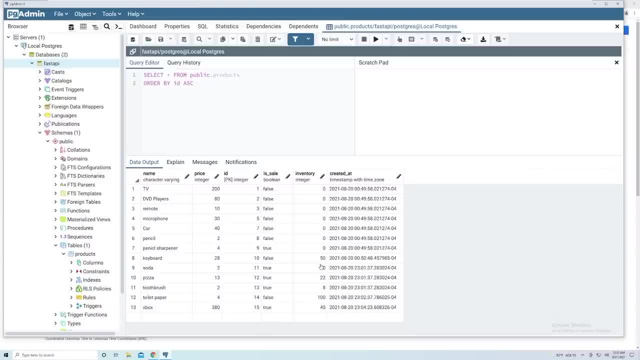 make sure that the inventory numbers vary enough and then try to create them at different times as well, if you can do that, That way when we actually go to make queries we can see a variety of different output, And that won't happen if you only have three to four entries. 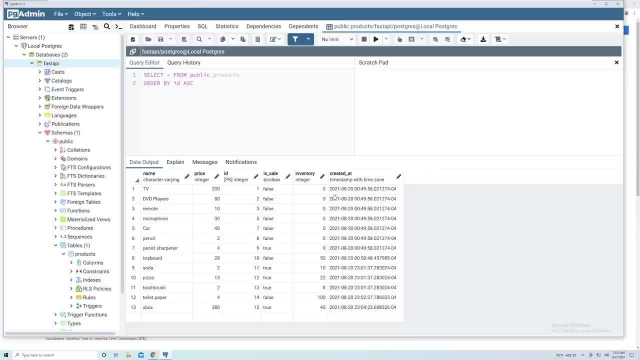 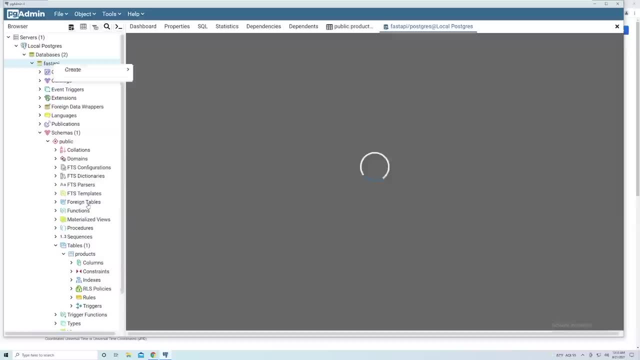 But once you do that, we should be ready to start our first query. And what we want to do is right click on your database- So my database is called fast API- and then select query tool. So that's going to open up a brand new tab. 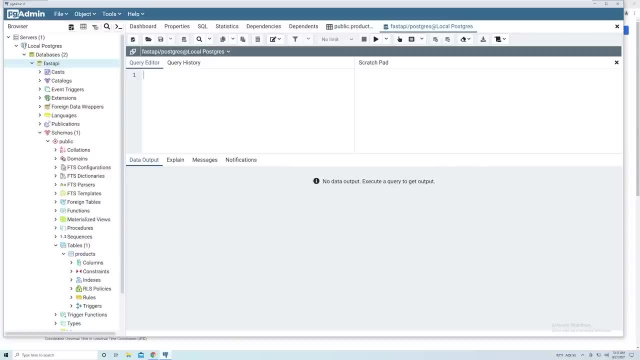 And what we can do is we can do a little bit of a search, And what we can do is we can do a little bit of a search, And what we can do is we can run our query from here. So here we type out our query. 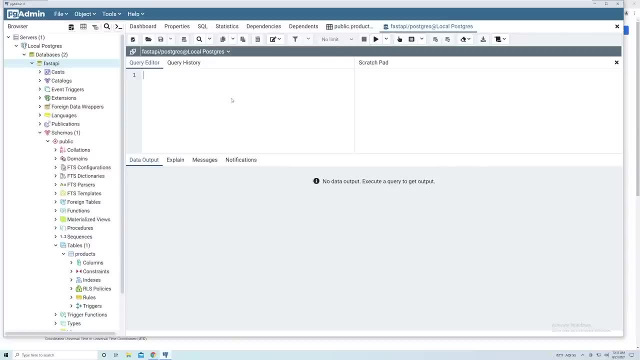 and then we just hit the play button and that's going to run our query. So how do we make a query within a SQL database? So first of all, let's start off with the most basic query. I'm going to type it out. 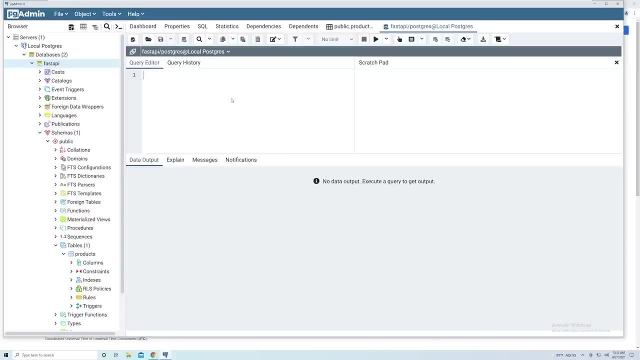 And then, after we type it out and run it, I'm going to explain to you exactly what each part of the command actually does. So here we'll do: select star from products colon. Then, once we've typed this out, what we can do is just hit the play button. 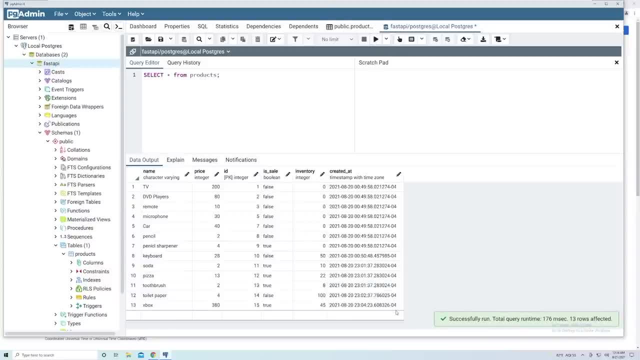 and let's see what happens. So this is going to run the query. We got the same output here saying that it successfully ran And it says 13 rows affected, And so what we can see here is it just printed out: every single entry within our products table. 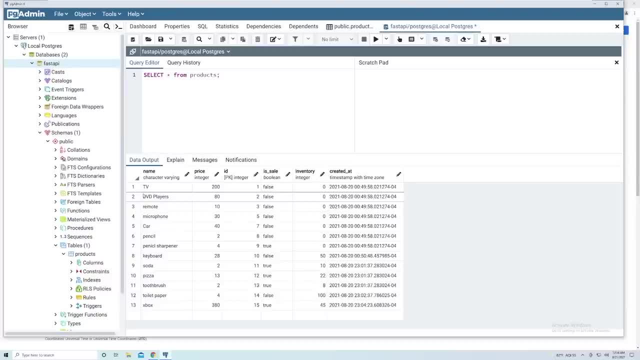 Now we only have one table, so it's essentially just dumping out the entire database. But if we had more tables you would see that this would only print out whatever was in our products table. So this command right here does one simple thing. 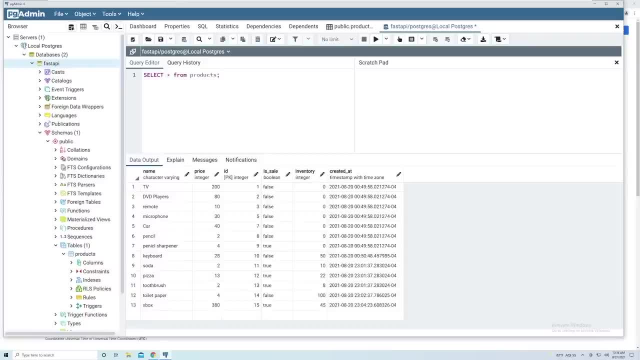 and that is. it's going to give us every single row within the products database. So let's actually break this down. So, first of all, we start this command with select. So we're basically saying, hey, I want to select these rows. 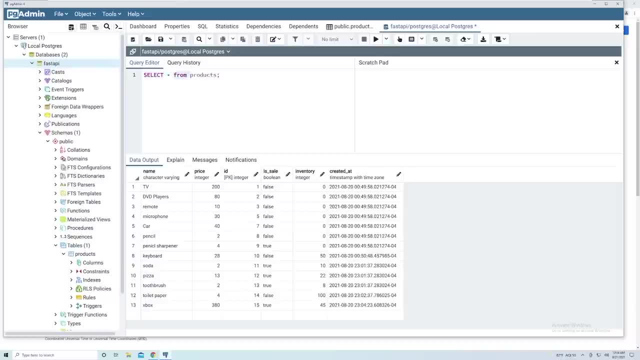 Ignore this for now. We're going to come back to this. And then what we do is we run from, and then products, And so you say what table you ultimately want to run this command for. So you say from, and then the table name. 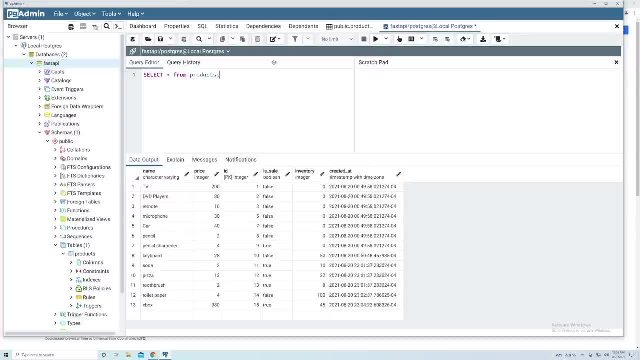 and then it's going to run that query against that table. If we had a table called users and we wanted to get every user, we could do select star from users, No different right. So it's just a matter Providing your specific table name. 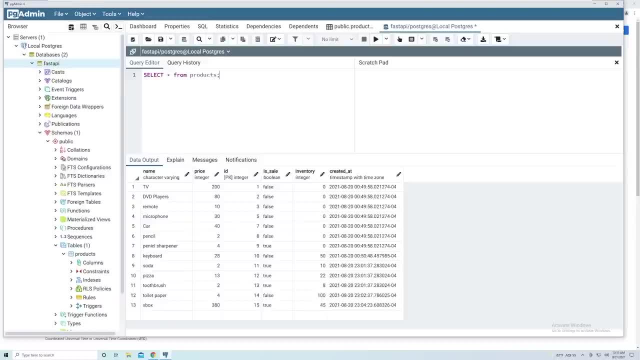 So every query is going to be with regards to some table, And the thing about SQL is every single command is going to end with a semicolon, So if I don't put the semicolon, it's not going to do anything. Well, in this case, it actually ended up working. 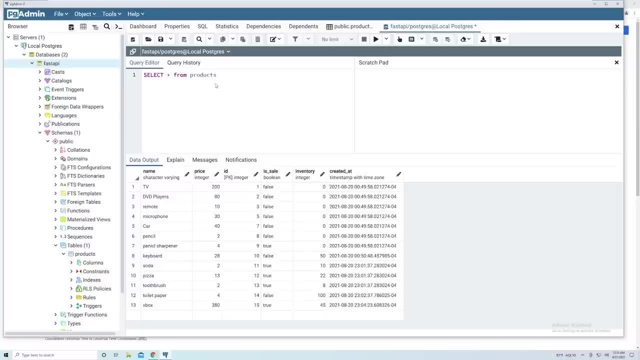 but that's just because we're using pgadmin. If you did this in the command line, it wouldn't have worked. So remember semicolon at the end of every command. Now let's talk about what this star, or asterisk, actually does. 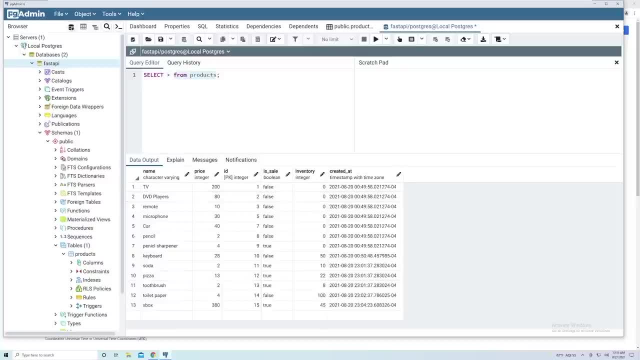 And so you could see, by default we get every row, and that's coming from this part of the command. But what does this do? Well, if you see, here we get every single column back from our table, And that's because we use the star here. 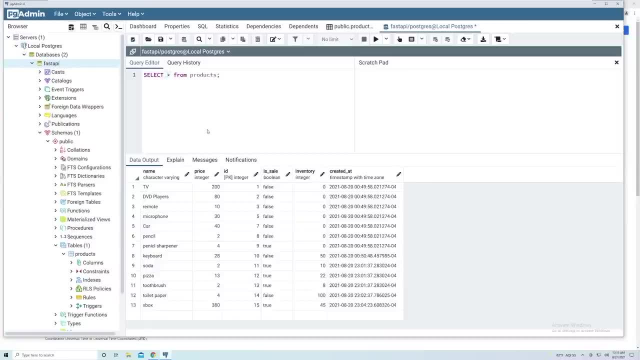 However, in an actual database, your tables could have 50 columns, maybe more. They could have a ton of columns, And if you're running a simple query to get you know some specific information, you may not want to get all of that data back. 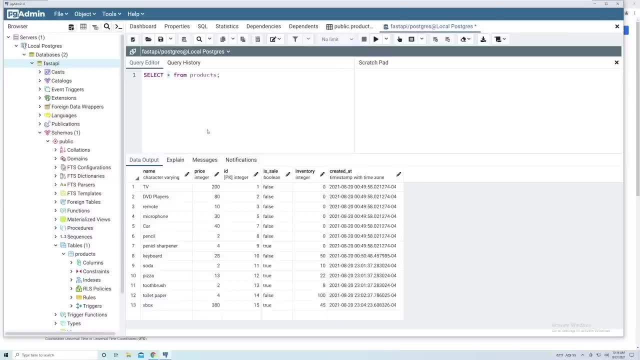 You may not care about most of the columns, You may only want one or two columns, And so we can filter out what columns we want, returned back for each row. So the star means I want every single column. So we got every single column that we defined for the table. 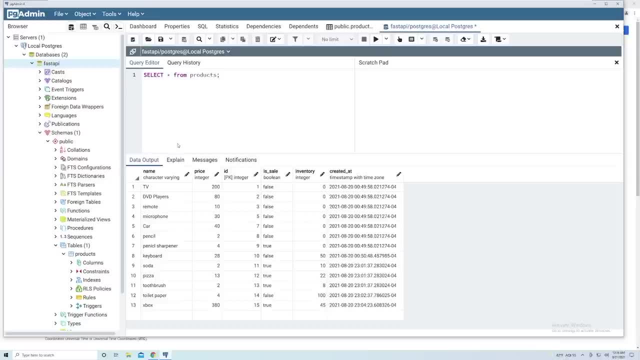 But if I wanted to run a query against the products table, but I only wanted a list of the different names of each product, I can specify just name, And so what this is going to do is this is going to grab just the name column from my products table. 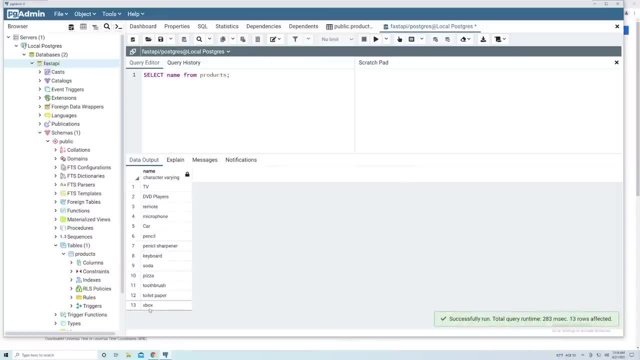 So if I run this again, you can see we got the same exact data, We got all 13 entries, but it only returned just the name column, And then we can add in as many columns as we want. So if I wanted the ID column as well and the price, 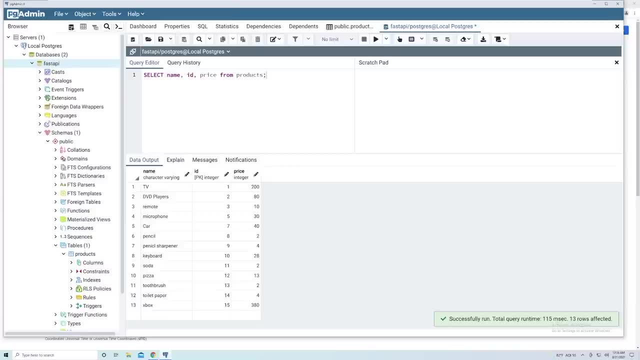 I can hit run. And so now we got the ID and the price, And what's really nice is it's going to line up with the order that I write them here. So if I want the ID first and then the name and then the price, 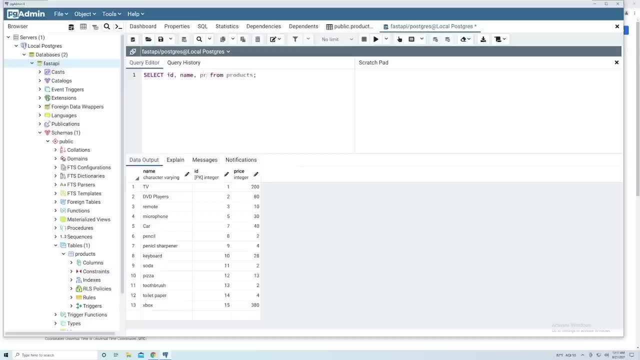 I could change this to ID name, price, And so now it's going to order it in that exact order. So we got ID name and price, But if you do a star, it's just going to return every single column. 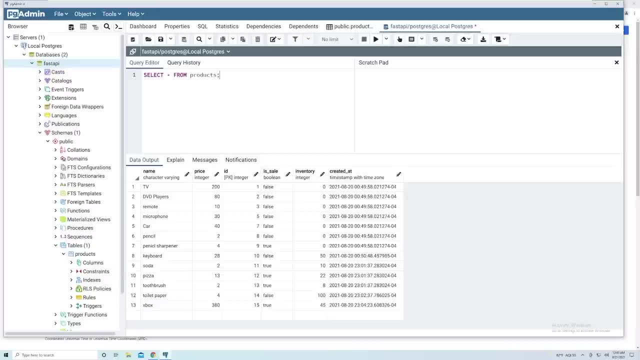 Now, before we dig any deeper into SQL and how to structure SQL commands, I want to talk about capitalization, And so you'll notice that when I ran this command, the word select and the word from is capitalized, And I want to make this very clear. 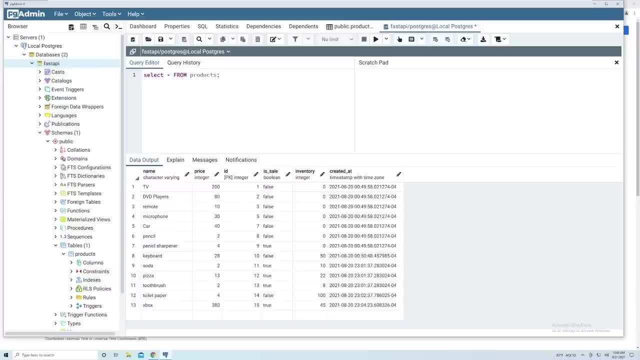 Capitalization doesn't matter. So if I make this lowercase and I make this lowercase as well, and then hit run, you'll see that everything works just fine as it did when it was capitalized. So capitalization doesn't matter. However, with a any SQL statement, we have two types of words. 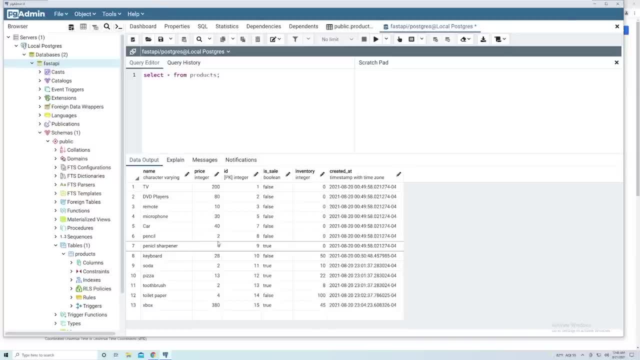 We've got SQL specific keywords, which is part of the SQL syntax, And then we have our user provided information, And so let's quickly talk about what those two things are. So the user provided information is keywords that I'm inputting in. 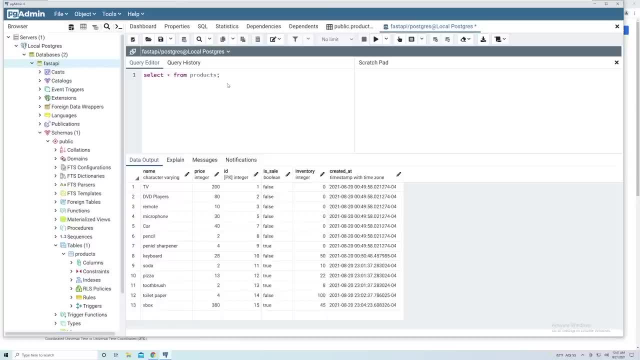 So I'm asking SQL or my Postgres database, I want the information from my products table, so I'm passing in this data and so that one you just you have to make sure you just match this up with whatever it's called within our table. 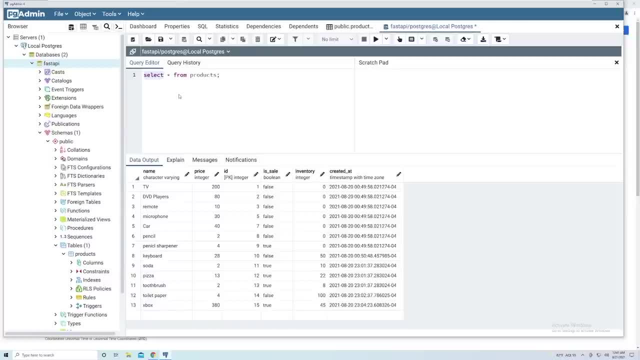 But all of the SQL specific words that I don't create that don't match up with anything in our database. right, those can be either capitalized or lowercase, It doesn't matter, It's not going to impact your SQL statement, but you'll see that best. 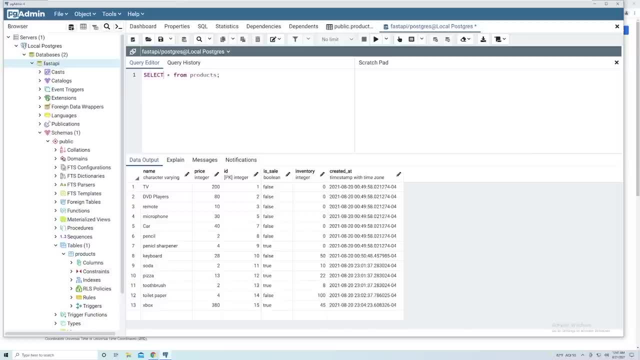 practice is to capitalize it, So we'll do capital select and then capital from, And the reason we do that is that we can much easier tell which parts of our SQL statement Is user provided information and what parts of our SQL statement is just basic. 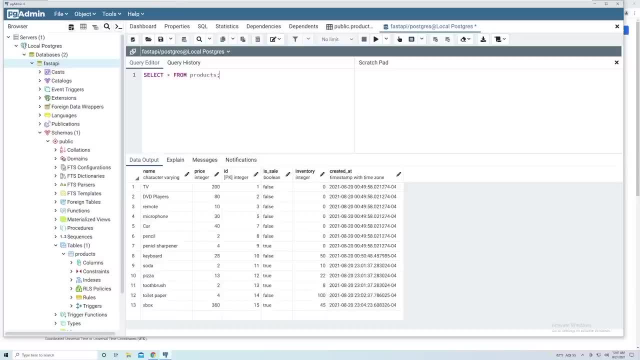 SQL keywords, So this just makes it a little bit easier to read. You may not notice the benefit of it now, but you'll see that these SQL commands can get really long. They can span multiple lines, And so having those keywords capitalized it makes it a little bit easier to. 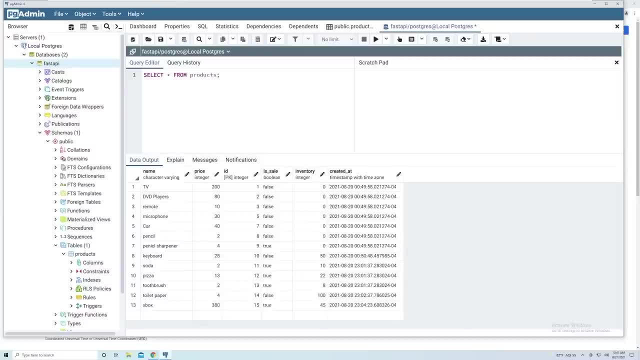 understand. But keep in mind, it doesn't actually impact how the command, how the SQL statement actually runs, So it doesn't matter. But if you want to follow along with what I do, I like to capitalize them Now with SQL. 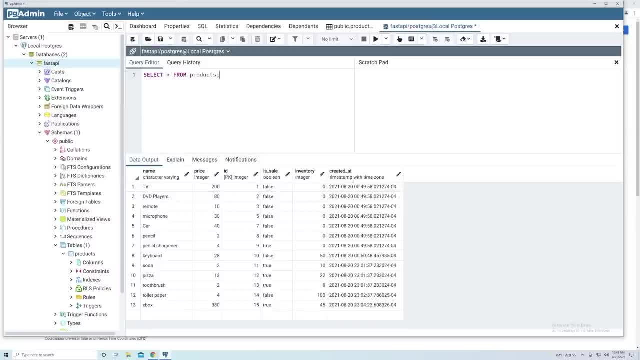 What we can do is when we perform a query we can rename any of these columns. So if we find that this name is a little inconvenient- and maybe you know, renaming it makes it a little bit easier on our back end code to better interpret- 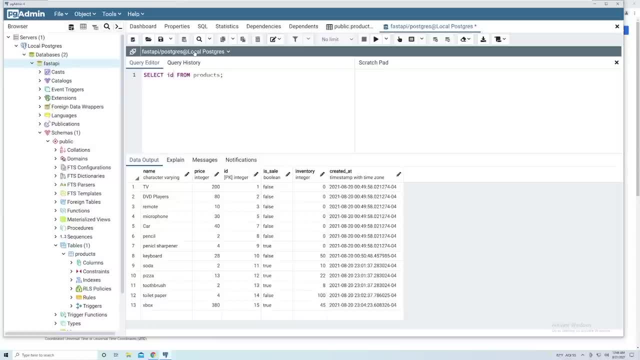 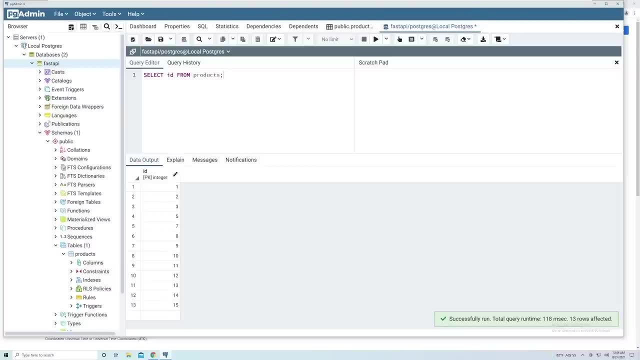 the data. we can pick any column we want and rename it. So let's say we're trying to fetch the ID column. I'm just going to run this. We can see we grab the ID column and it's named ID. But let's say, this confuses our back end because we're retrieving, maybe data from. 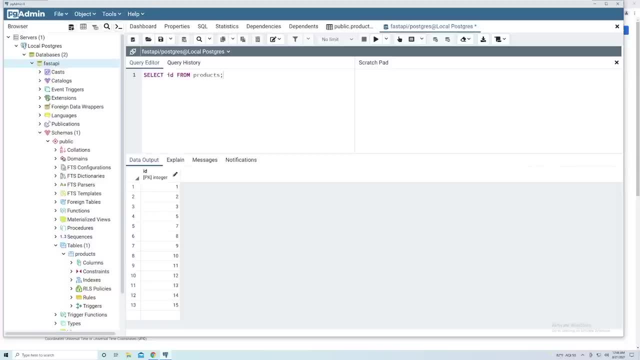 another database that also, you know, for users or something, And then we also have an ID field And we don't want them to get mixed up. I can rename this column and we can rename it by using the as keyword. So I say ID as and then specify the new name. 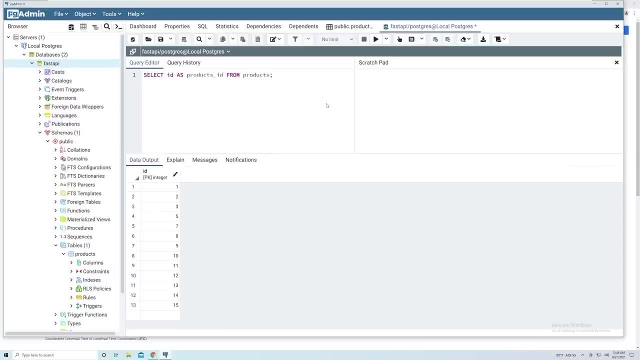 So I can name this products underscore ID. But now if I run this, we could see that the column is now products underscore ID instead of just ID, And I can do this for any and as many columns as I want. So if I wanted to rename the is sale column, I can save it as on sale. 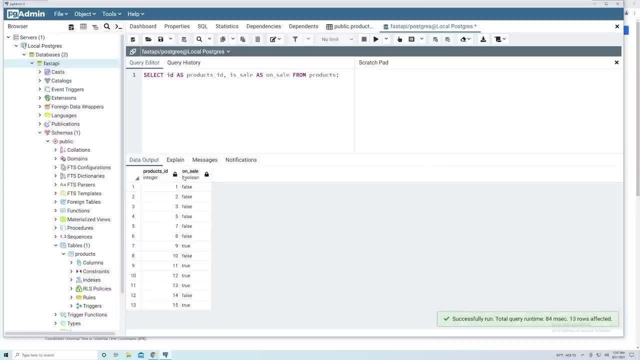 And so there you go, guys. it's really as simple as that, Keep in mind. I kind of continued with my normal SQL format of capitalizing the SQL specific keywords, just because it makes it a little bit easier to read, All right, so let's clean this up a bit. 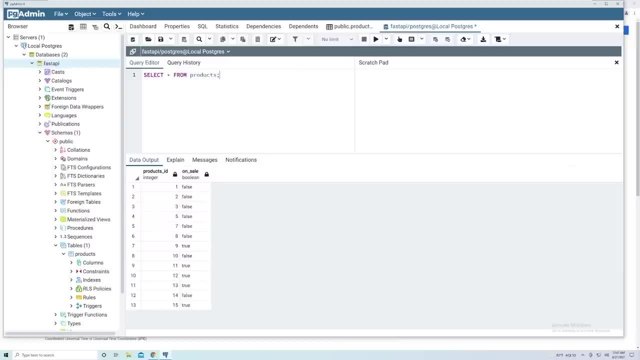 I'm just going to change this back to star so that we can retrieve every single column. is going to run that, just to make sure nothing's broken. And so till now we've been retrieving every single entry in the table, and that's because we've provided no filter criteria. 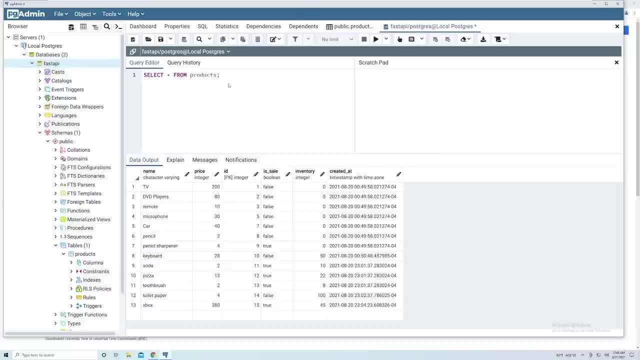 No filter Condition. So let's figure out how we can filter the specific rows that we want based off a certain criteria. So let's say I want to match all entries that have a specific ID of something right, And we know there's only going to be one entry that has a specific ID because the ID field 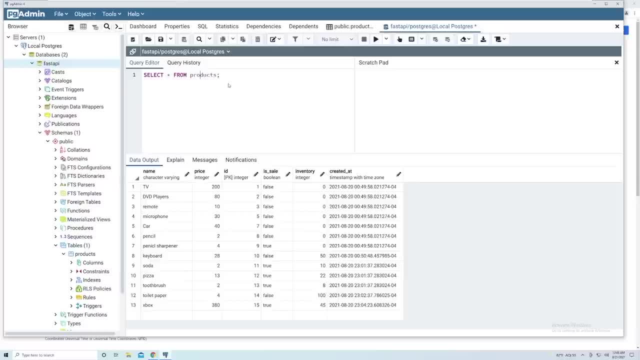 is a primary key, So we know that two different items can't have the same exact ID. but you'll see, one of the more common tasks when it comes to working with databases is retrieving a, a row, based off of a specific ID. So you know, a lot of times our back end will be like: hey, I want you to retrieve. 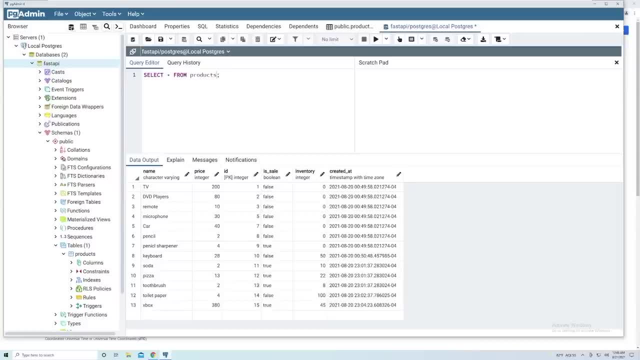 the product with an ID of 10.. So how do we do that? Easy, We add the keyword where then we specify the column that we're interested in, that we want to match on. So we're going to use the ID column, And then we say ID equals, and then we pass in the value. 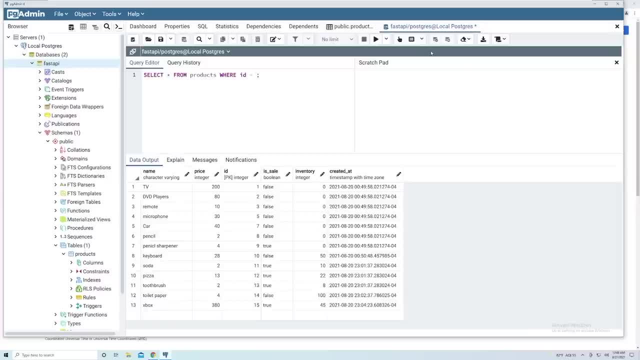 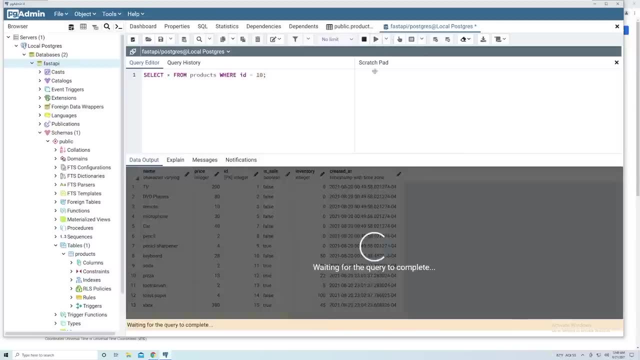 It's really is that simple. So if I want the ID of And so if I want to get the product with an ID of 10, I just pass in 10 and remember to make sure you have the semicolon at the end: hit run. 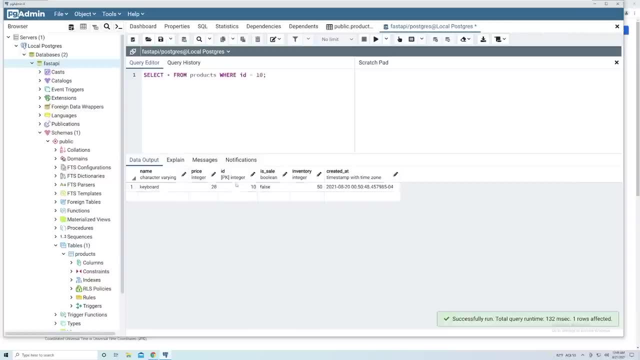 And look at that. We've now got our product that has the ID of 10. And then keep in mind, just like we did before, we can filter down based off of just the fields we want. So if we want just the ID and the name, we can do that and it should work just fine. 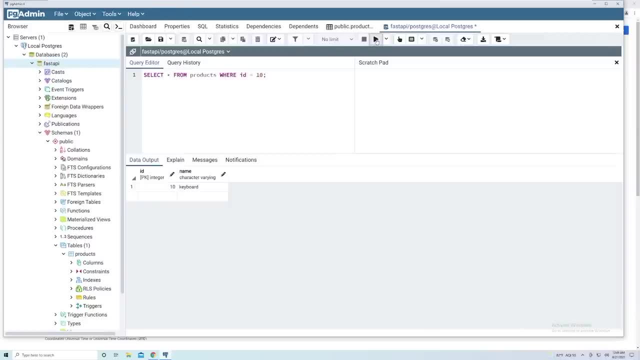 We'll change this back and run that, And so we got that. If we want to grab the idea of product and an idea of three, run that, And so now we get the product with an idea of three. But what's nice about this is that we can choose any column to match on. 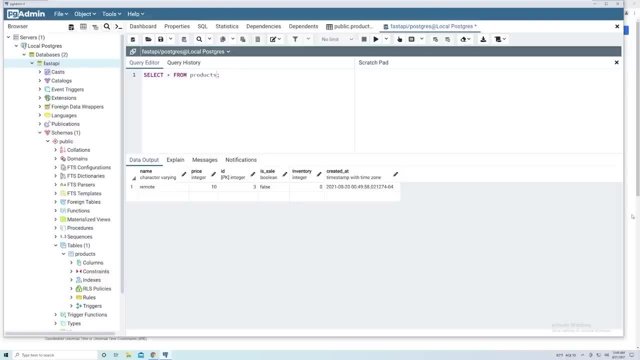 So let's say that I first dump everything so I could just see what I've got. And let's say I want to match on any product that has an inventory of zero. So that's basically saying, like which products do we not have inventory of, so that maybe? 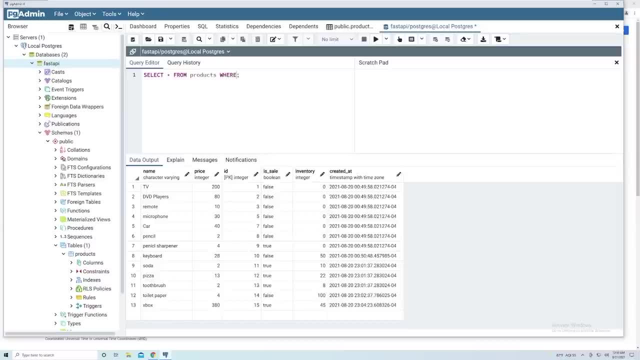 we can place an order. Well, we can just say where, And once again I'm capitalizing the SQL keywords. I can say where: OK, Inventory equals zero. And so now we've got a list of products where we need to place an order. 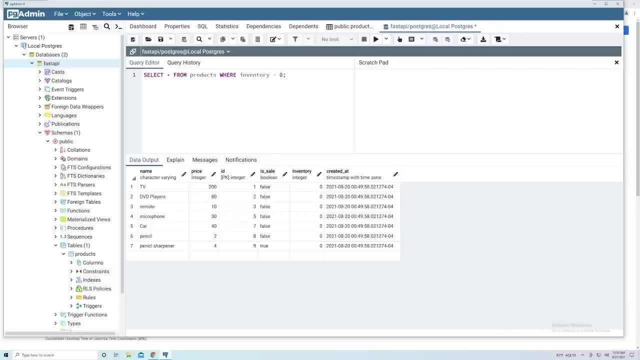 It really is as simple as that. Now, working with numbers, you just place the number. So any column that uses integers or floats or anything like that, you could just say, equals that. However, if you want to match based off of name, the name column, it's going to be a. 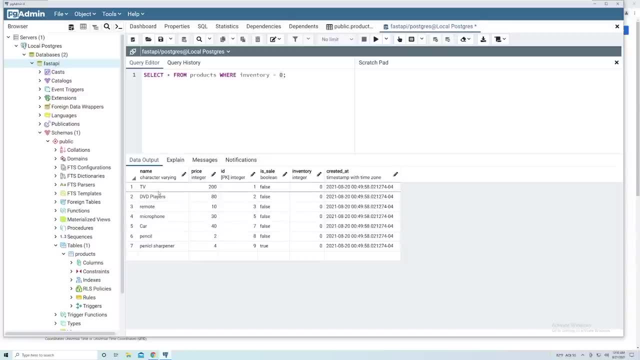 little bit different, because the name column uses varying characters or text or what would be a string in Python, And so for those, what we have to do is, first of all, we'll use the column name equals, but we have to wrap it in quotes, single quotes to be specific. 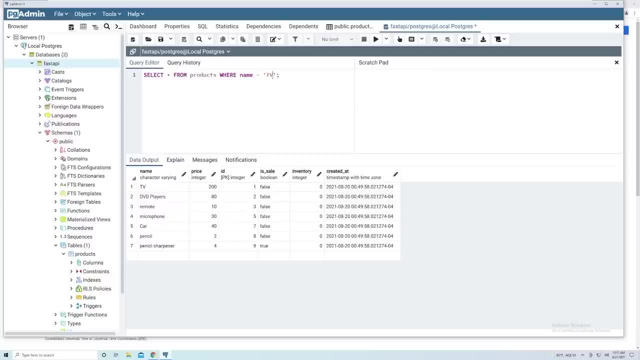 So if I want to get the product with the name of TV, I have to put in single quotes, search for it, And then now we get that. But keep that in mind, because if you remove the quotes I believe you should get an error. 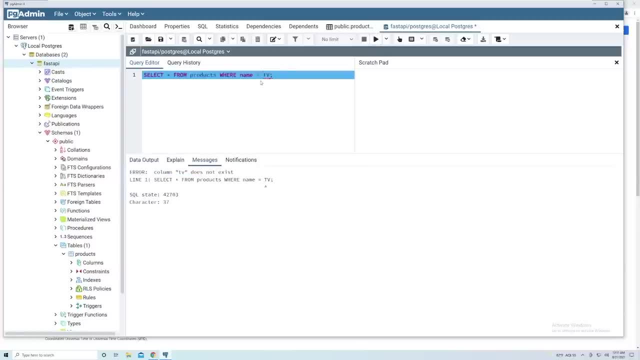 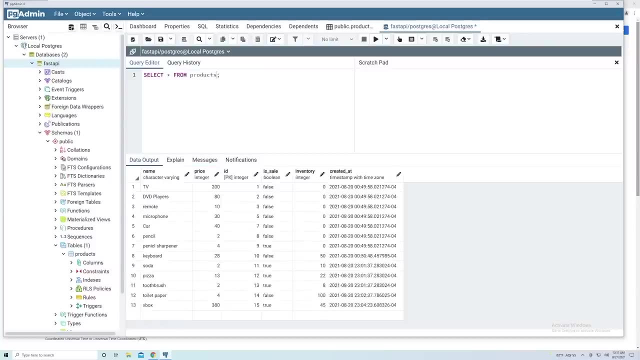 Yep, And you do get an error. So just make sure, when it comes to working with varying characters or any kind of text, you want to wrap it in quotes Now. Now, just like with most programming languages, we do have operators. 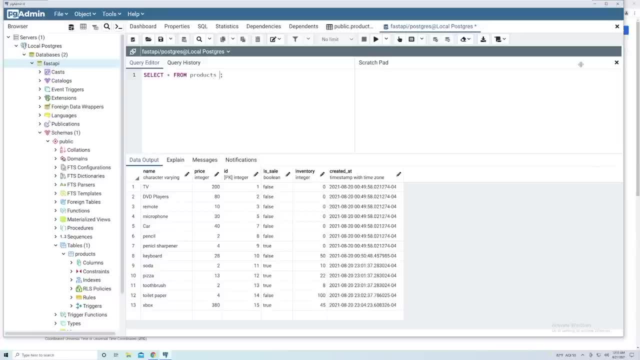 And so till now we've just been working with the equals operator. So if I need to get you know any product that has a price of, you know, 20, I would just say where price equals 20 and I don't look. it looks like I don't actually have. 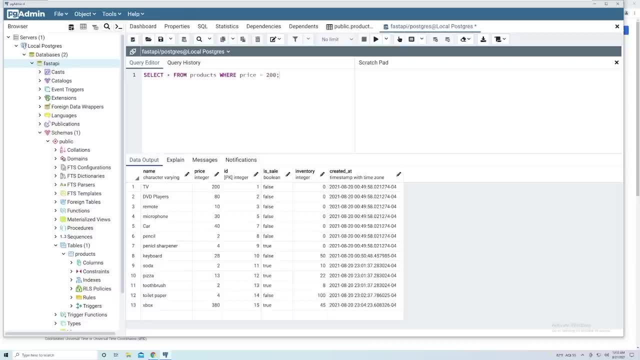 any items with the price of 20.. So I'm just going to do 200, because I see that the TV is 200. if we run that, it works just fine. However, what if, instead of doing this, I want to retrieve all of the items that have? 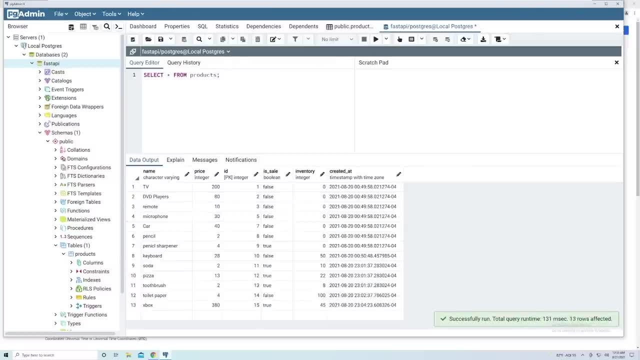 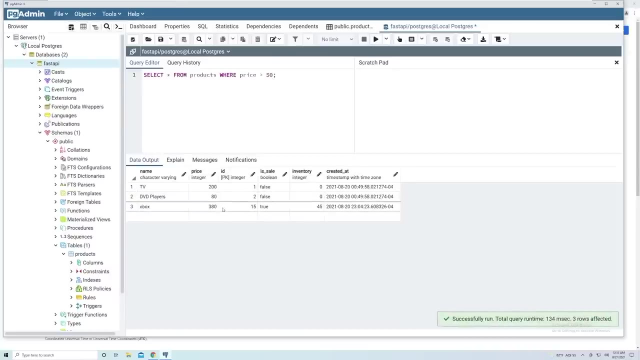 a price of greater than 50. How do I do that? Well, it really is fundamentally no different than how we do in Python. So I could say where and I'll say price is, and then we have greater than 50. So this is going to grab any item. that's basically 51 or higher. 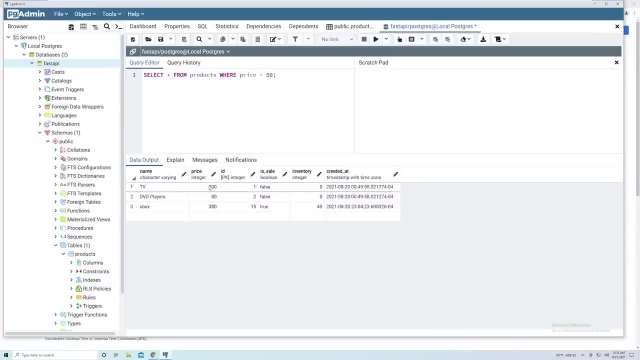 And it's not inclusive, so it doesn't include 50. And so now look it, looks like it grabbed all of the items that cost more than 50 bucks. But if I wanted to say greater than or equal to 50, I can say just greater than or equal. 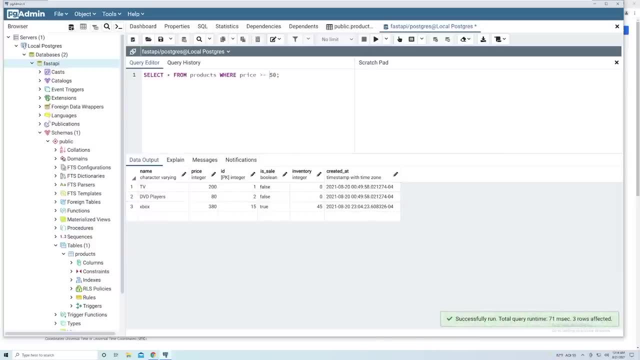 to 50.. If I run this, we can see once again. it works just fine, But I don't have any products that are priced at 50. So I'll try this again with just 80.. So we'll say greater than 80.. 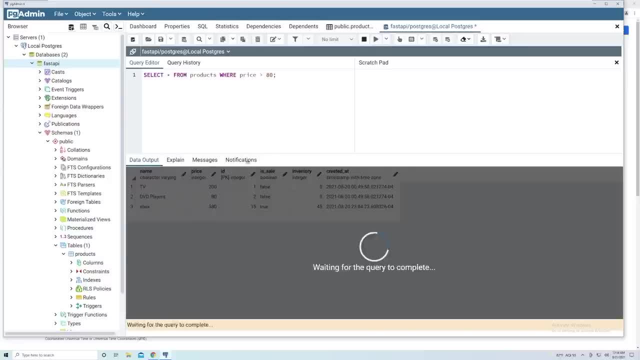 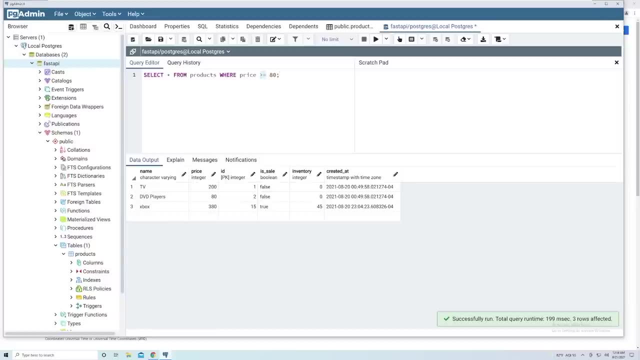 It should not return this one, because 80 is not greater than 80. But we can see the 80 is gone. But then if I do greater than or equal to, we can see the 80 is back And we get the same thing with the less than and less than equal to. so I could say less. 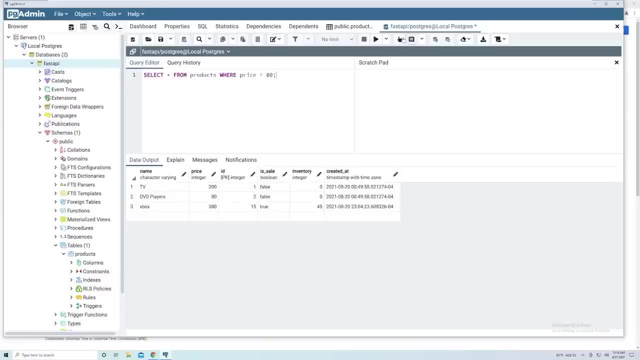 than 80. And I could say less than or equal to 80 as well. And the last operator that I want to discuss is the not operator. So if I wanted to grab any product that does not have a inventory of zero, I can say where. 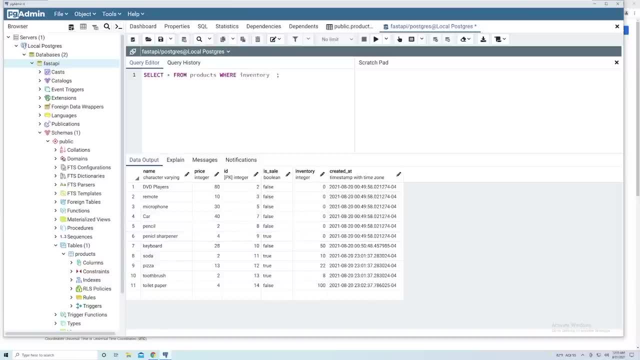 inventory And we have two different ways of doing this. I can say not equals. So this is kind of the similar syntax that you see in some other programming languages- not Python, but other programming languages. I could say not equals And then zero. this is going to give me every product that we do have adequate stock for. 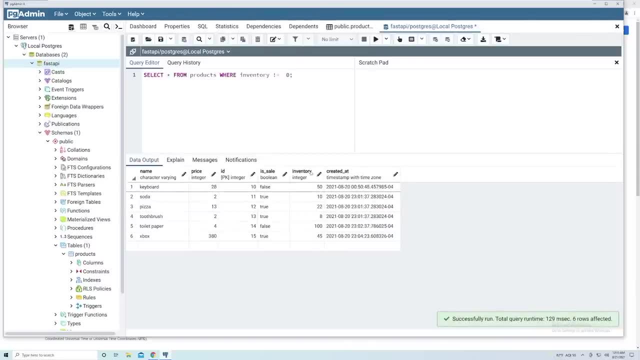 And so now we see we get no columns are sorry, no rows with an inventory of zero. But we can also use this syntax: So the greater than sorry, the less than, and then the greater than we run that we should get the same exact result. 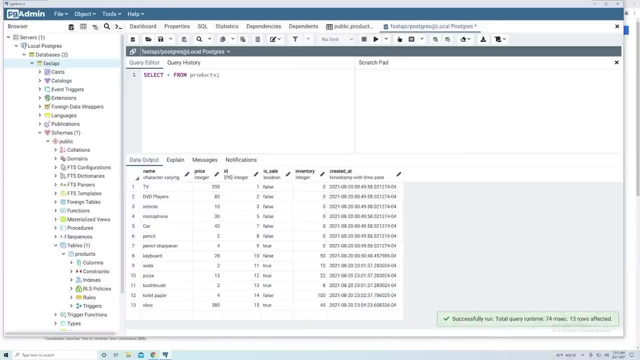 Alright, so let's move on to performing multiple operators. So let's say: I want to grab any item that we have inventory of, So any, any item that has an inventory greater than zero that also costs more than $10.. How could we do that? 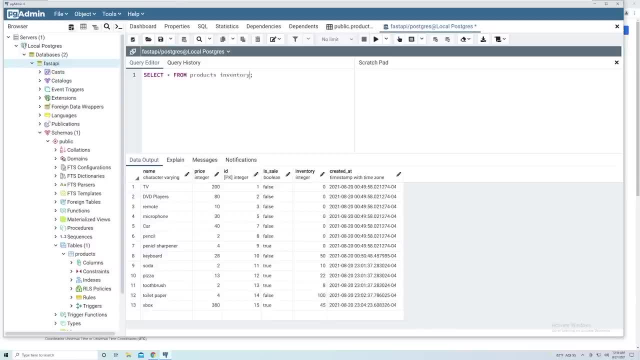 And I'm sure you guys can probably take a guess at this, but we'll do inventory greater than zero. And then how do we add that next statement where we say greater than- I forget what I said- greater than 20.. So we could just say, and simple as that, we do and and then we pass in the next criteria. 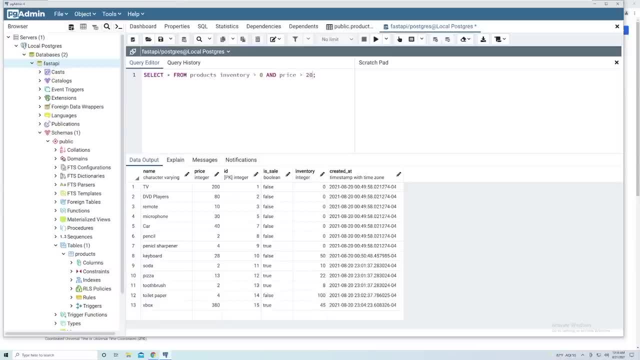 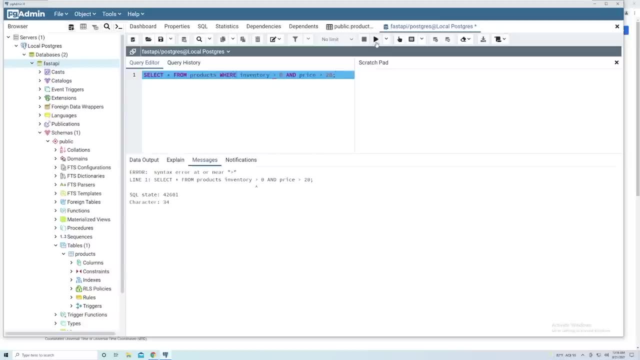 will say: and price is greater than 20.. Let's try that out. And I realized I forgot the where keyword here, So that's why it's throwing an error. And so now we got every single product that has a inventory greater than zero and a price. 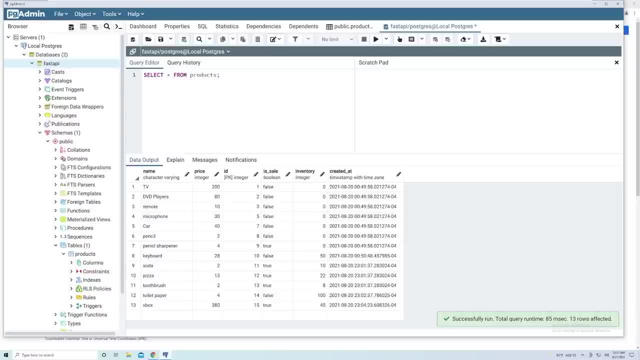 of greater than 20.. And just like with an and operator, we also have an or operator, And so if I want to see any product that is either greater than $100, or less than 20, I can say where where price is greater than 100. 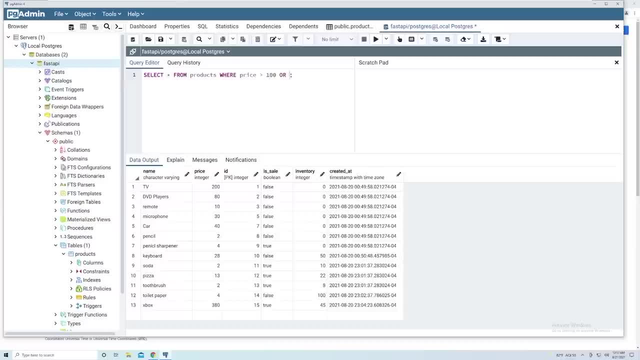 Or price is less than 20.. And so now we can use two criterias, And as long as it matches one, one or both of the criterias, it's going to return that result. All right, let's clean this up a bit. 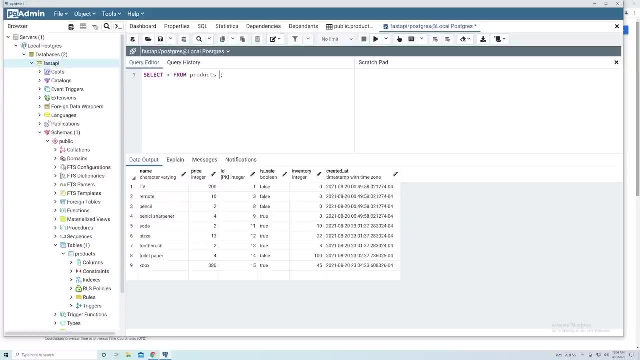 And let's say I want to retrieve products with an ID of one, two and three. How would I do that? Well, I can do where where ID equals one, And then we'd have to do an or statement, And then we'd say ID equals two or ID equals three. we run this. it should grab just those. 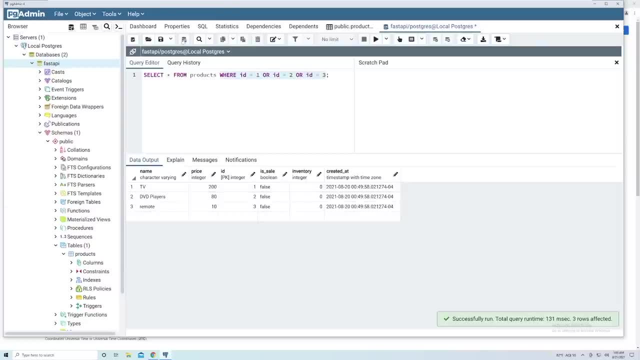 three items. Now there's another way to perform this kind of operation, And instead of using all of these ID equals one, ID equals two and then just combining them with or statements, we can use the in operator. So let me explain how the in operator works. 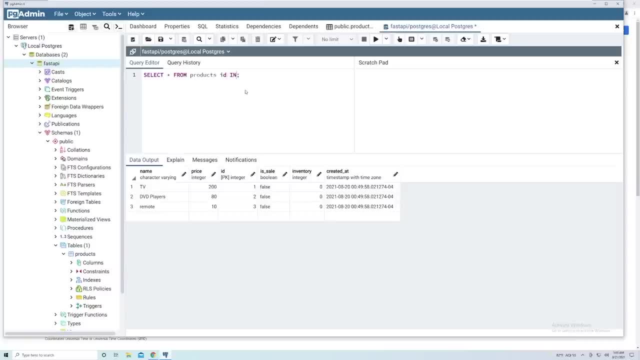 What we can do is we can say ID in And then we can provide a list of values. So I can say one, two and three, And once again I forgot the where keyword, And so if you run this you can see that we got the three items. 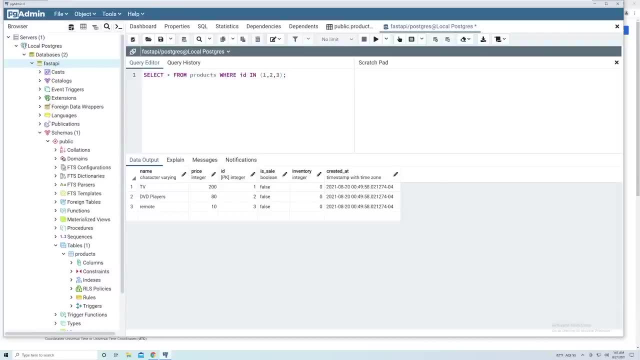 And you can see that that's way more readable instead of having to type out that entire command. And let me show you the previous command. I shouldn't have deleted it, So I'm going to use a scratch pad just to show you guys. 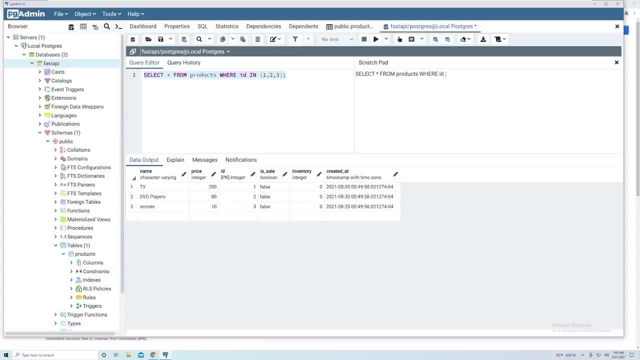 And so before we did where ID equals one or ID equals three, And then we can see that we got the three items, And then we can see that we got the three items, And then we can see that we got the three items. 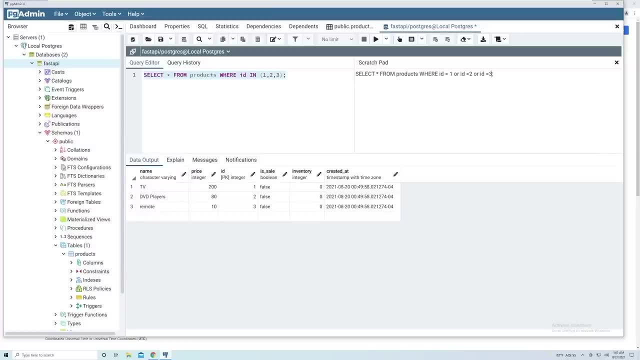 So ID equals two, or ID equals three. So which one do you think is more readable? So both of them do the same exact thing. However, one's a little bit easier to read And it cuts down on the number of keywords that you have to type. 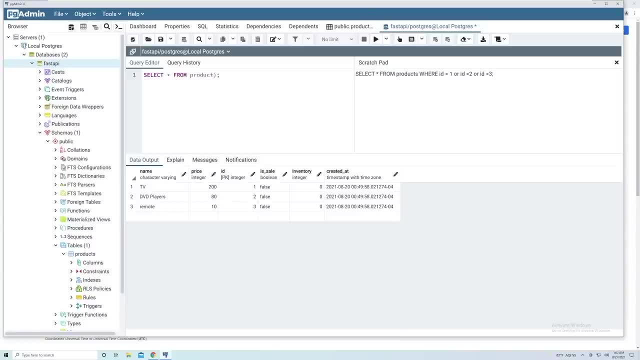 Now we, before we proceed any further, I'm just going to retrieve all my databases- sorry, all my entries once again, And what I'm going to do is I'm going to add a few items, And so all of these items are going to be named. 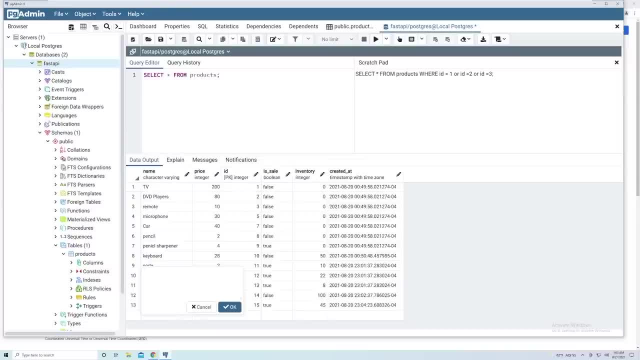 very specifically. So I've got a TV items And so I'm going to call, I'm going to create one called TV blue, And then let me give this a price, And then everything else I can leave default, And I'm going to create a TV red And then a TV yellow And I'm going to save. 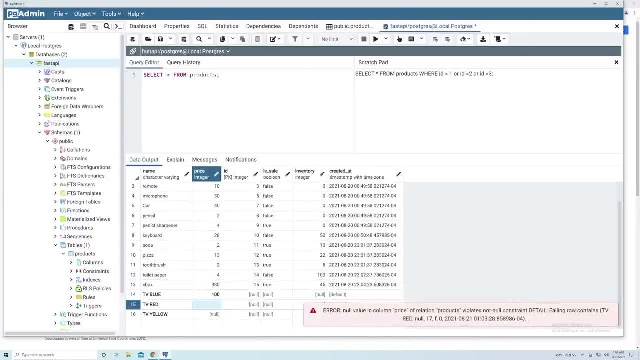 these to our database And I forgot to give it a price. We'll just say all of them cost actually, let's give them different prices. So this one, 200, yellow. no one likes anything that's yellow, So I'll give it a value of 50.. And we'll save to our database. All right. 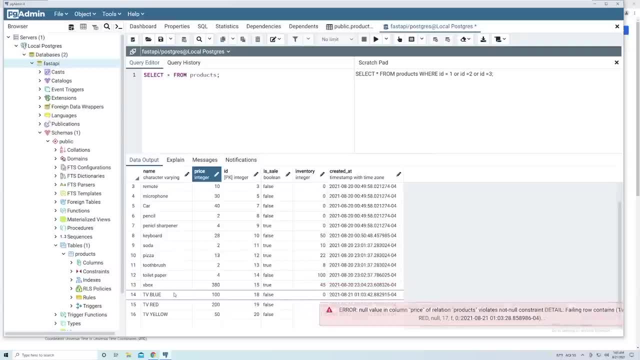 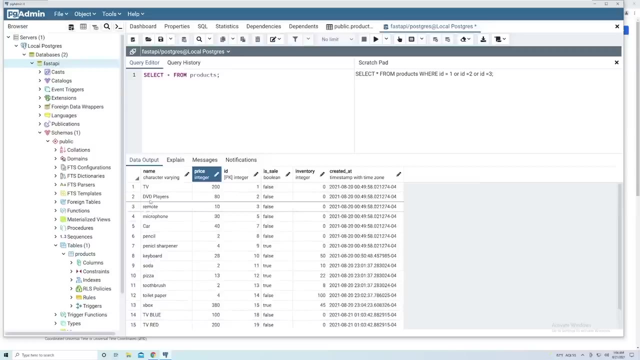 so that's in our database now And we know how to filter based off of items And we can use the where keyword and we can do it for even columns that are based off of characters, like the name column. So let's say that I want to retrieve everything, all of my TV, So this TV. 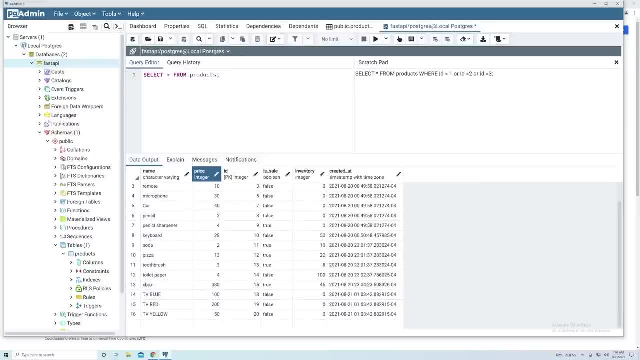 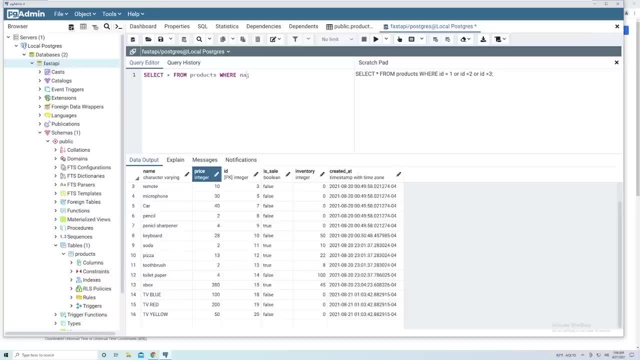 Well, we can use our like operator So we could say where name like, and then what we can do is we can pass in something very specific, So we pass in the text that we want, But then we can start using things that are kind of like regular expressions, like we have in Python. So I could say TV, and then 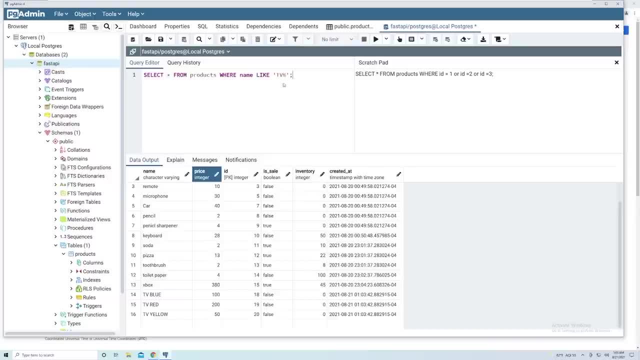 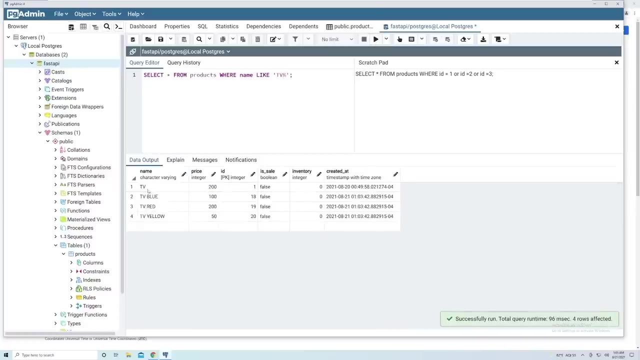 percent sign And what this is saying is that I want to grab every row that has a name that starts with TV, and then the percent sign means any random characters afterwards. So this is just saying I want any product that has a name that starts with TV. So if I run this, you can see that we were 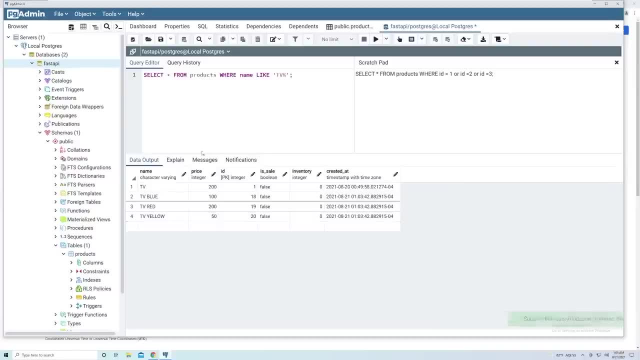 able to grab all the TV. So it's very similar to regular expressions, And if I remove this and instead, just you know, add in the letter A, this is going to return all of my products that start with the letter A And I. 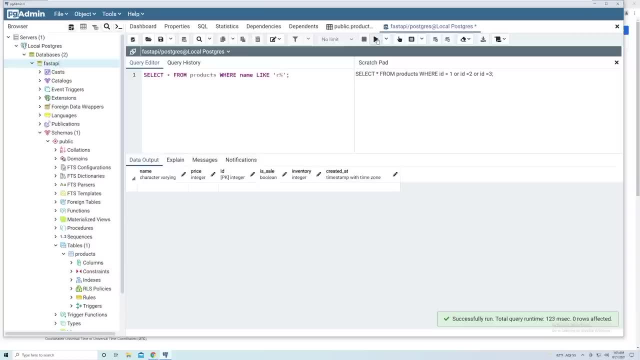 don't have anything. But if I change this I know I have one product that starts with an R. So if I try that, you can see that we get the remote And we can also flip this. So I can say, you know. 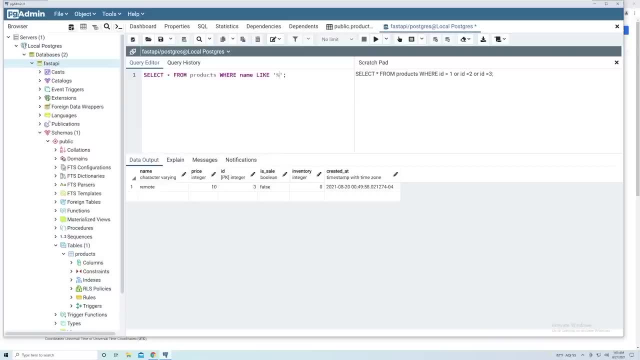 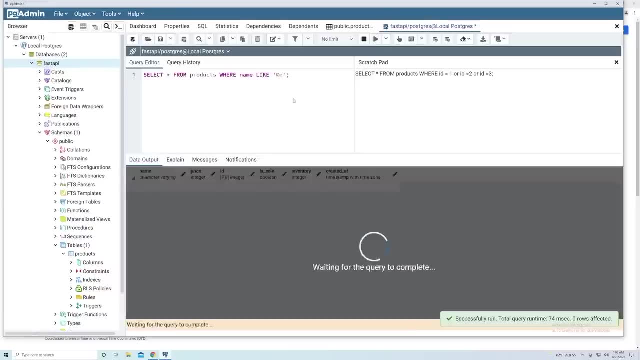 percent sign and then pass in some letters at the end. So if I want to grab anything that ends in the letter n, I can run that. it looks like I've got nothing that ends in the letter N, Maybe II, and so now we get all of the items that end in an II. 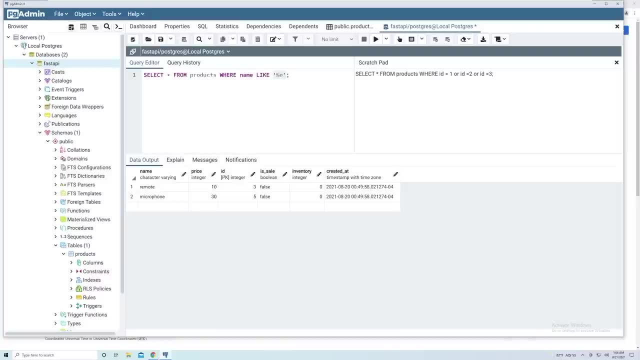 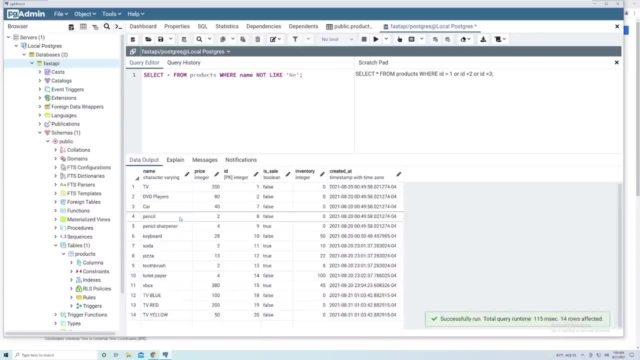 And then we also have the ability to do the opposite. So this matches anything that ends in an e. but if I want to get every line that doesn't end in that e, I can say not, but that's just going give me the opposite. So that's going to give me every row except for those two rows, And what we. 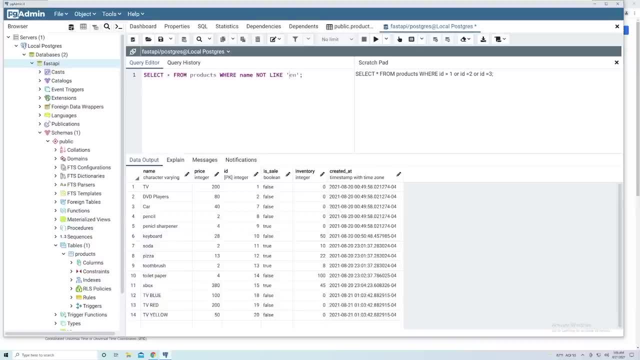 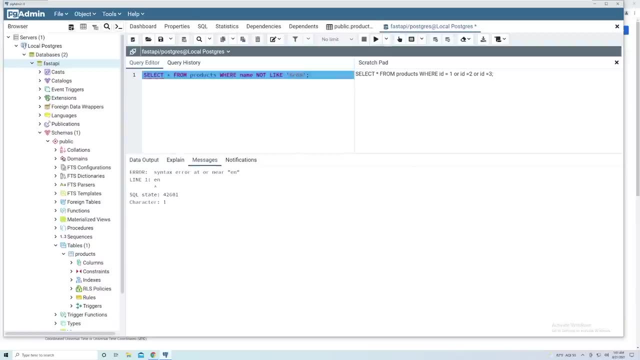 can also do is if I want to get any line that has the letter en somewhere in the name, I can do the percent sign before and after, And so two characters anywhere in the name. So if I run this and it looks like I got an error And I'm 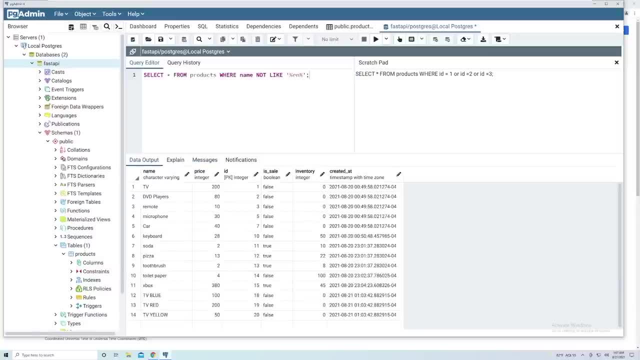 not sure what happened there, But I changed this. I just deleted and retyped it, And so now it no longer gives me an error. So I'm not really sure why that happened. Could be a bug of some kind, or maybe there's a typo- I didn't see. But this is going to grab any text that has the letters en. 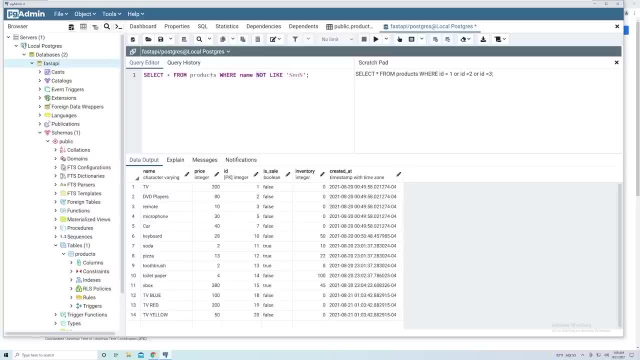 and then it can have any characters before, any characters after, And then, since we have the not operator, then it's going to do the exact opposite. But then I can also remove this so I can grab any lines that match just this, And then it looks like: once again I get the same exact error. 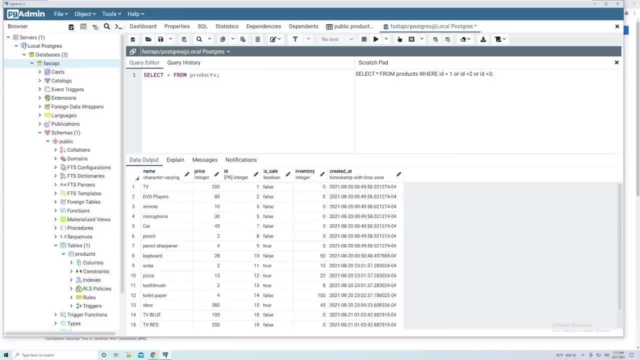 Okay, there we go. Now, when we make a query to our Postgres database, we can also specify how we want to order the results. Now, by default, it looks like it's just going based off of the ID, but it's not necessarily going to be like that, And so it's better to actually tell. 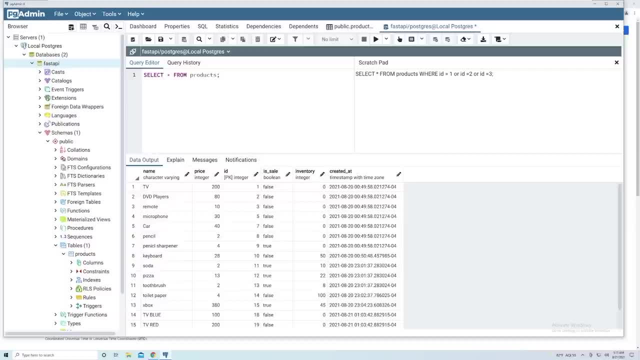 Postgres how you want to order the products. So in this case I've got an error here, So I'm going to go ahead and add an error here, And then I'm going to go ahead and add an error here, And then I'm going to go ahead and add an error here, And then 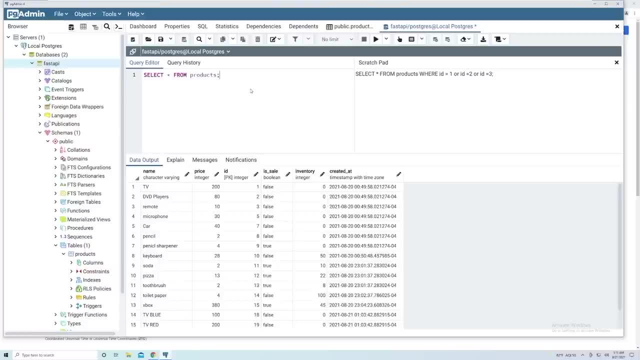 no filter criteria. I'm just returning everything And let's say I want to filter or order the the products that are returned based off of price. So if I say order by, I can then specify the price column. So let's see what happens when I run this Right. we could see that it looks like it starts. 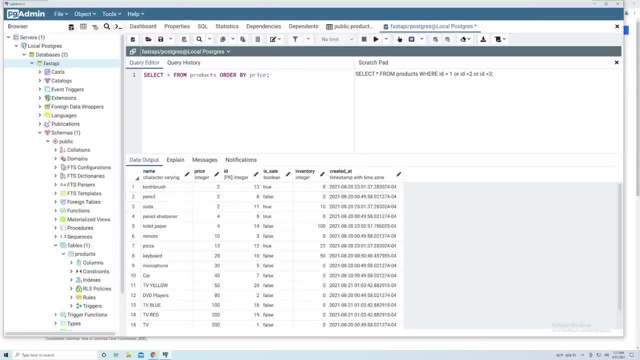 at the lowest price and then works its way up. So by default, when you specify the order by keyword and then specify the column, it does it in an ascending order, And so you could specify the order at which you want to go the direction, I guess, by saying ASC. 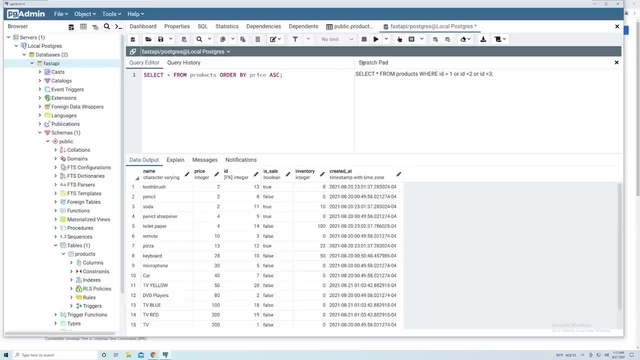 So this means ascending. So this shouldn't change anything because Postgres by default is going to always do it in an ascending order. So if I run this, nothing changes. However, if I want to do this in a descending order, I can say DSC for descending. So now it's going to start, at the most. 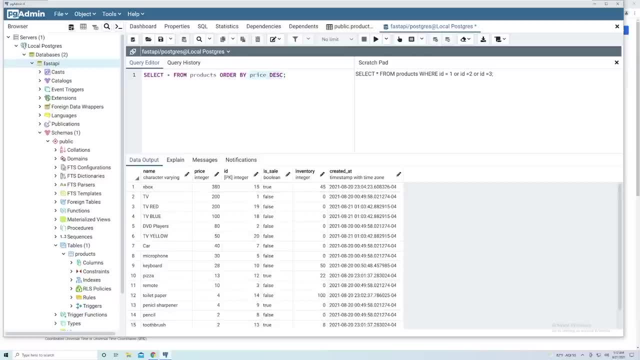 expensive price and then work its way down. Now let's change this And let's say we want to order by inventory And I want to see which products we have the most expensive. So let's say we want to have the most stuff. So I'll say inventory and then descending, because we want to start at the 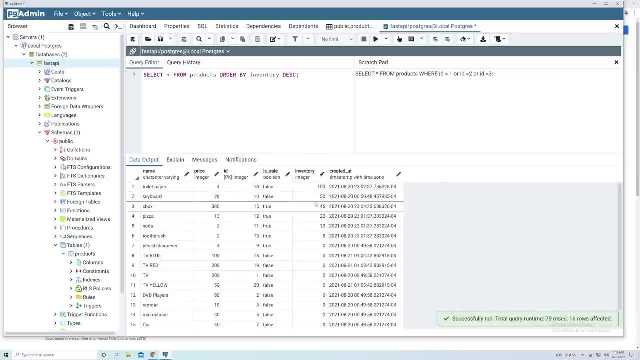 highest value and work our way down. So I'll run this And then we can see it starts at the highest one and then works its way down. But we've got a whole bunch of zeros And let's say that between these guys I also want to specify a tiebreaker of some kind. we can also specify the order. 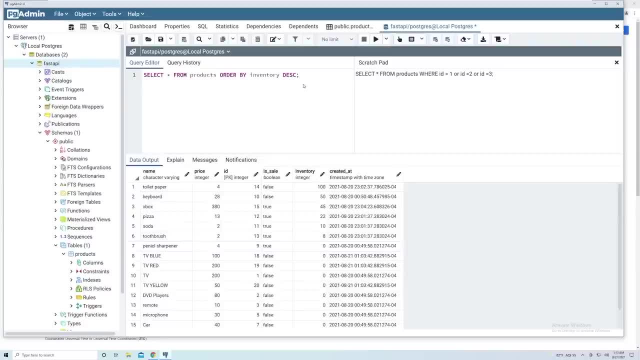 using a second column for these tiebreakers, So I can pass in another column, And so let's say that anytime there's a tie, I wanted to then order it by let's say price. So I'll say price And then we'll say the cheapest price. So ascending Now. 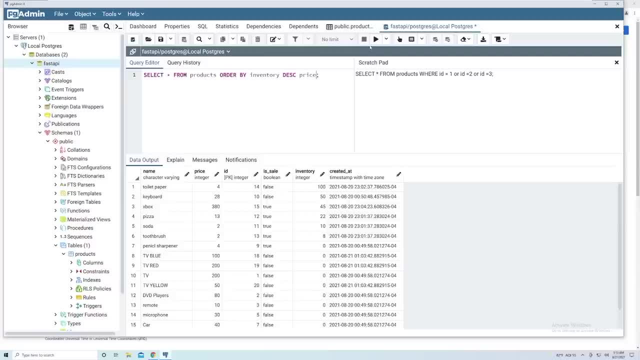 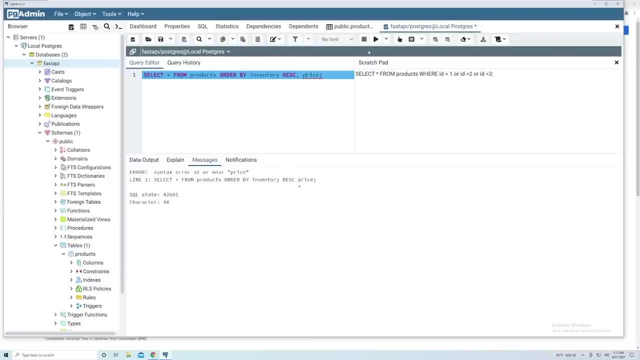 ascending is always the default, So we can just delete that keyword. And so let's run this now. And I forgot to put a comma, So after each column that you want to sort by, you have to do a comma, And so now we got all of our data, And so let's take a look and see if this actually works. So 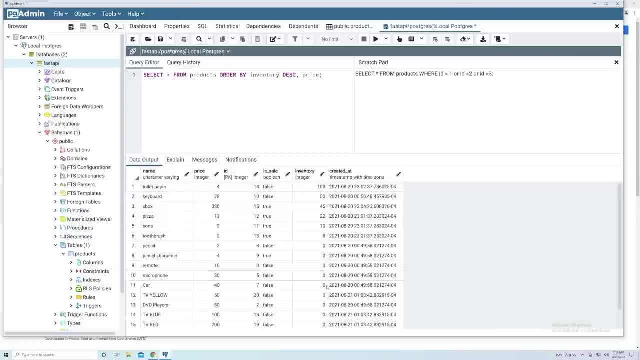 we can see we're sorting based off of inventory, then we get down to zeros. These are all tied. So we take a look at the second column that we pass. In this case we're looking at the cheapest price And so if we see the first one looks like the cheapest price is. 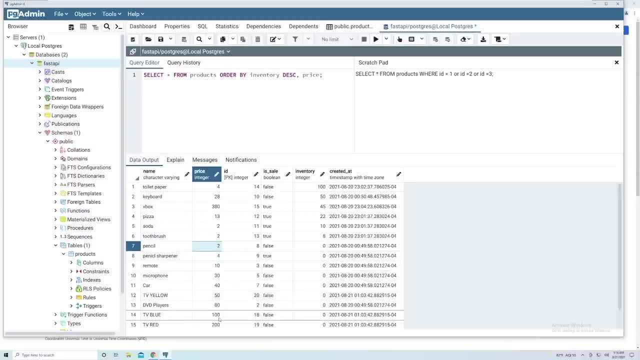 two, then it goes up to 410, 3040, 5080, 100, 200.. And you can pass in as many columns as you want For your sorting criteria. you don't have to just stick with two, And it's really just a matter of. 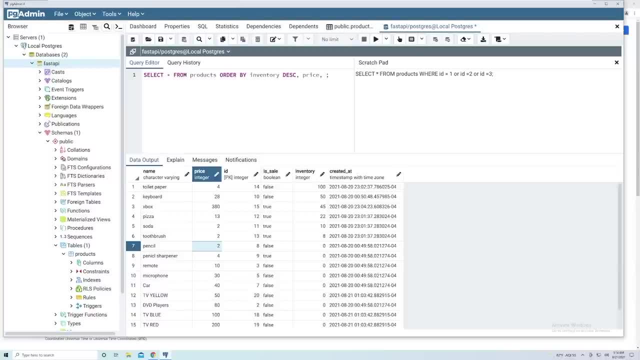 doing a comma and then passing in the next column, and then whatever the criteria is, And you'll see that one of the common things to do is, let's say, we want to get the most recent products. Well, I think it makes sense to just sort based off created. So that's. 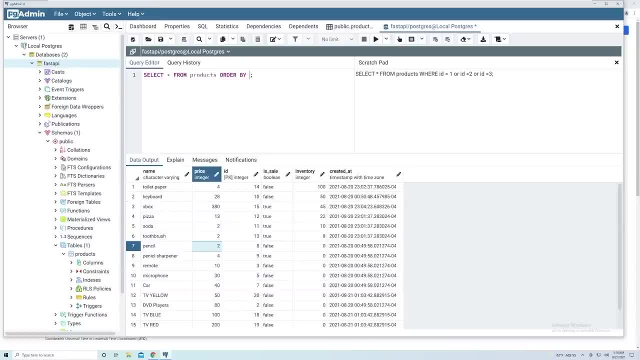 the timestamp for when the product was created. So let's see what was the most recent products that were put into our database. we can just say created, underscore at: And what order do you think we need? Do we need ascending or descending? If you don't know, think about it. And if you still, 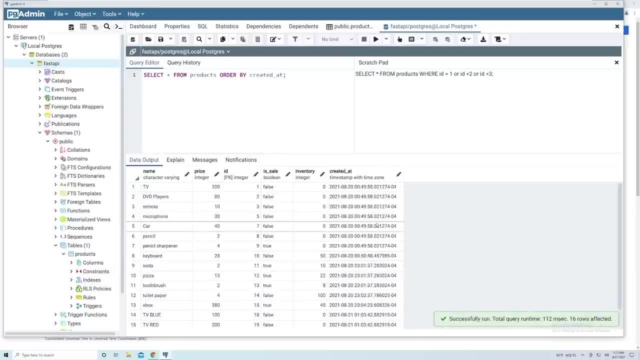 don't know, test it out. That's the easiest way to find out. So we can see that the first one is ascending. So when it's ascending, we can see that there's a one. at 820 is created a 20. And then 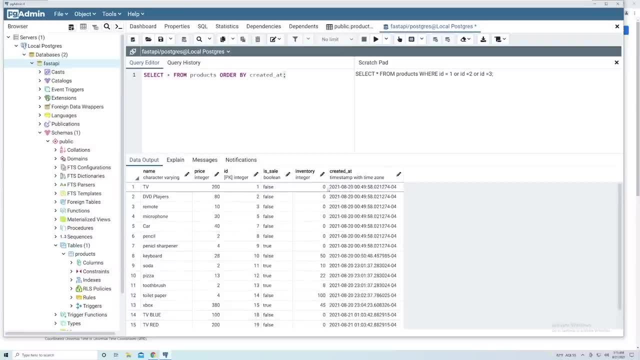 the bottom ones are created a 21.. So it looks like this starts off with the oldest one and then works its way up to the most recent one, because that has a later date. you think of the later date as a higher value. So if we want the- you know, the most recent products first, we would do descending. 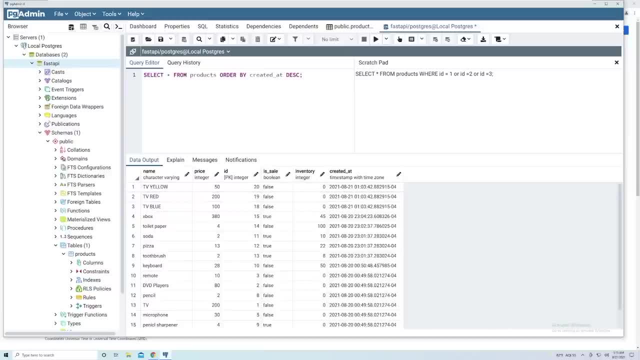 And so now we've got the most recent products And with this order, with the sorting property- remember, we can just chain this on to any SQL statement- So if I also wanted to, you know, get all of the products that have a price of greater than 20,. 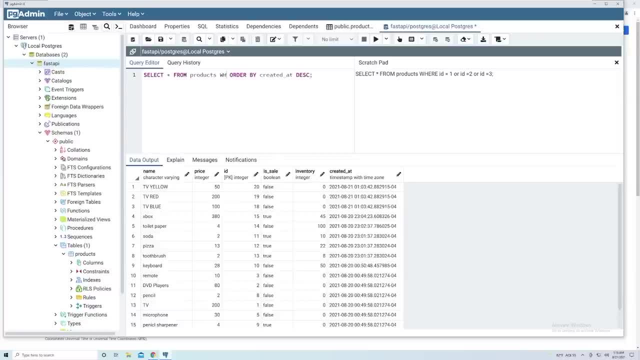 and then sort it by something. I can just specify my where keyword and say where price is greater than 20.. And then for all of those results I want to order by who was most recently created. we'll search that, And so there you go. 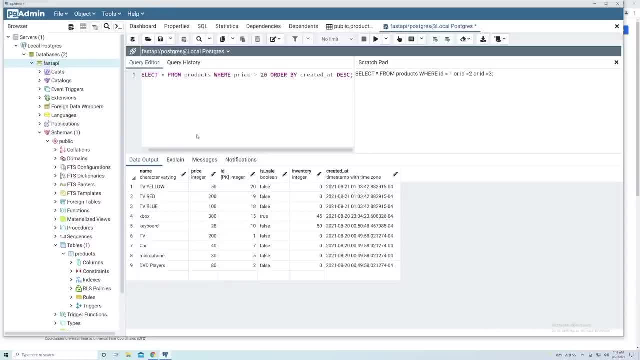 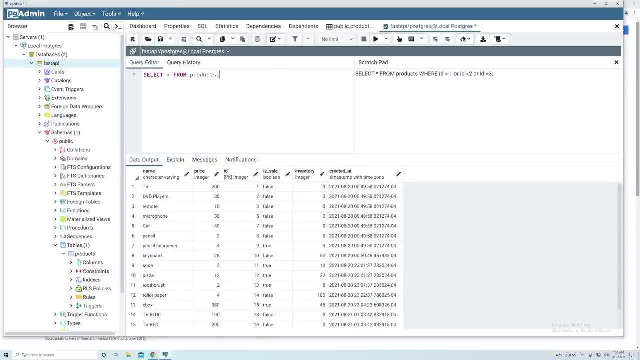 And so that's the great part about SQL, is you'll just keep chaining these different SQL keywords to filter out the exact data in the exact order that you want. Now, in an actual production environment, our tables could have millions, 10s of millions. 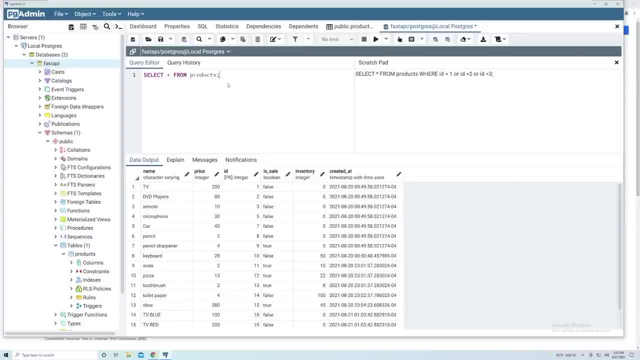 hundreds of millions of rows, And so it would never make sense to just perform a query like this where we just dump everything, because then all of a sudden we're asking our database to send back 100 million rows, And that's just unacceptable. And our software that we're using to even send the 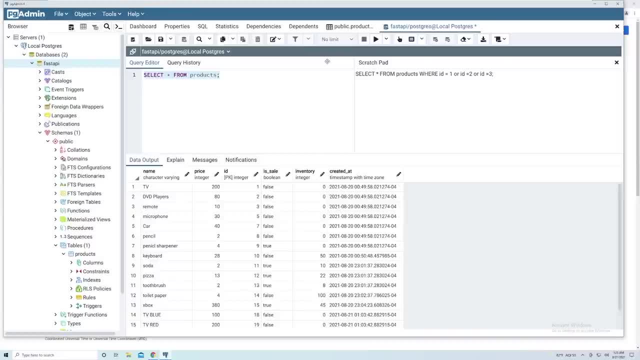 data to that database is not going to be able to handle that, And so usually you want to provide a limit of some kind. So you may want to say, Hey, I want to grab, you know, the first 10 rows that. 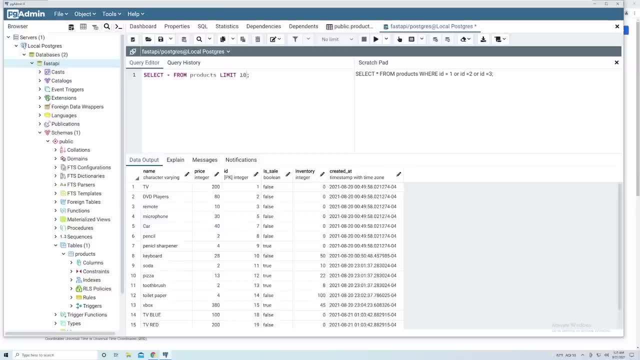 match this criteria. Well, we can do that by using the limit keyword. So we say limit and then pass in the number of rows that you want. So if I run that, you can see that we get 10 rows by lower. 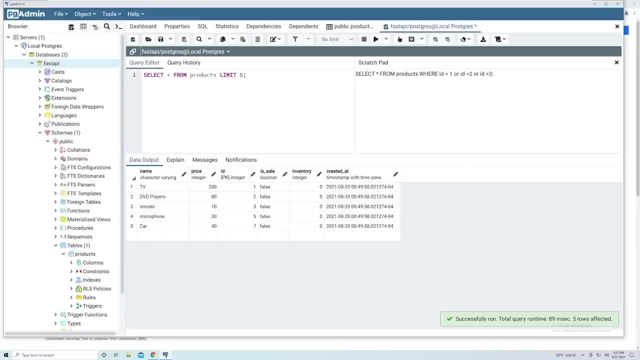 this to five. we can get this. we can get five rows And you can chain this on to any SQL expression. So let's say I wanted to grab all of the products of greater than 10.. If I search that, you can see I get 10 results. And let's say I want to limit this. 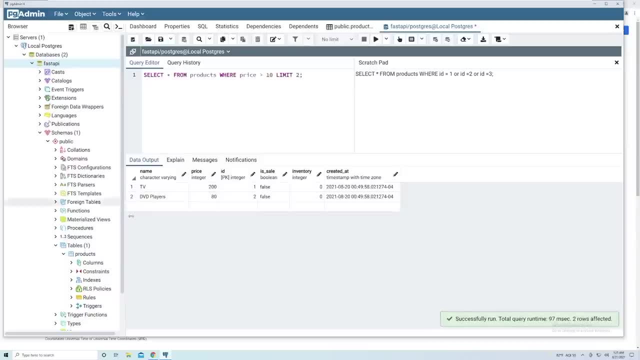 to only the first two results. So if I hit that, you can see that now I get two results. So all the keywords that we're covering, including the order by any of the filter expressions, we can just keep chaining on to our SQL statement to further specify exactly the data that we want Now with limit. 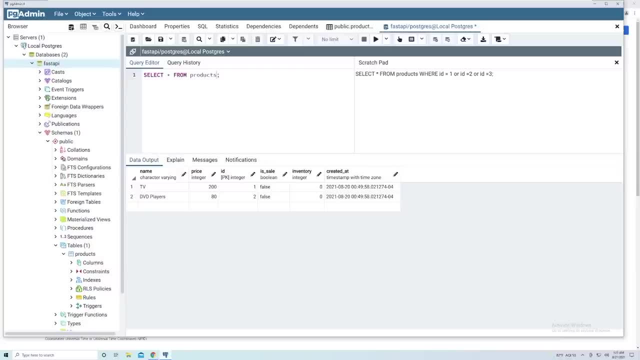 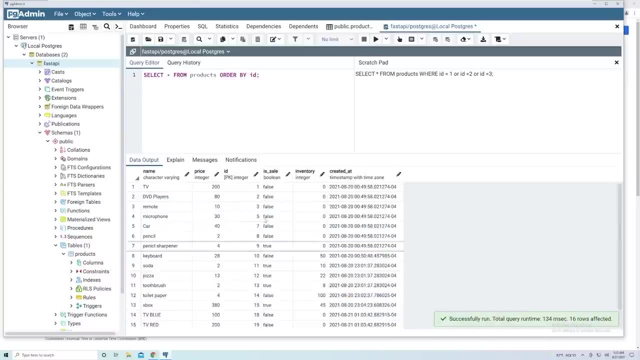 there's another keyword that I want to cover, And so let's say that I want to grab all products and I want to order by ID, Right, so it's going to return it like it normally does, and it's ordered by ID. 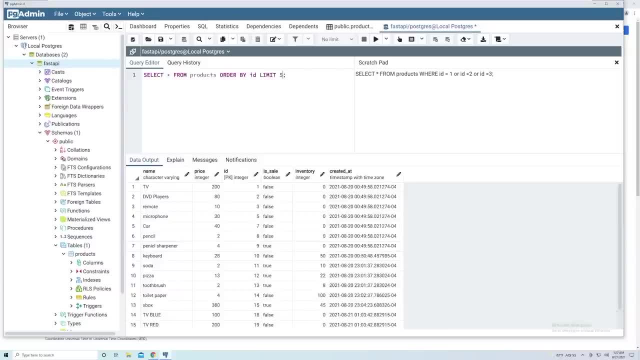 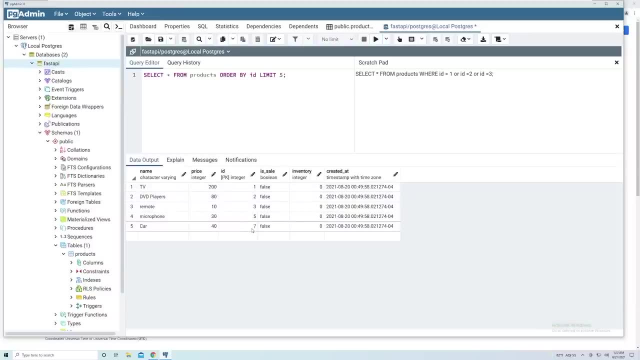 And let's say I want to set the limit to be five And now we get products with an ID of 123, five and seven. Do I not have a ID of six? I'm just curious actually, So let me cut this out for a second. I just want to see if there's an ID of six. There isn't an ID of six. 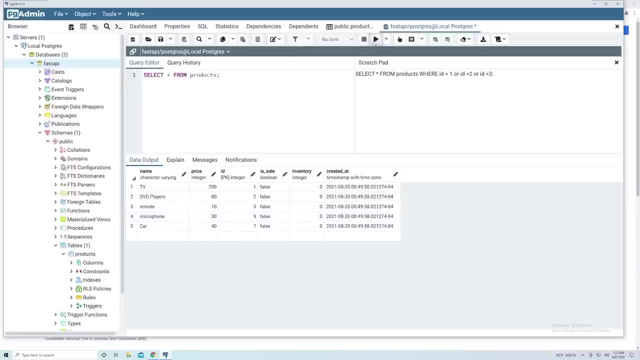 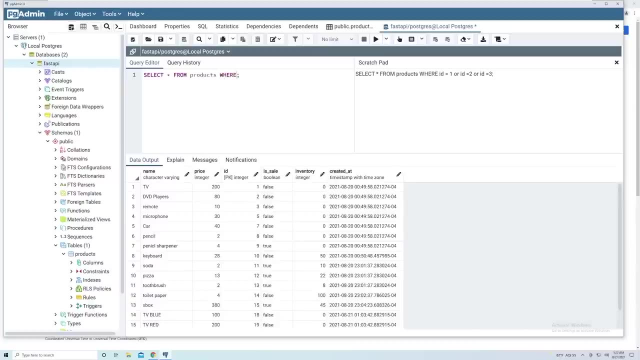 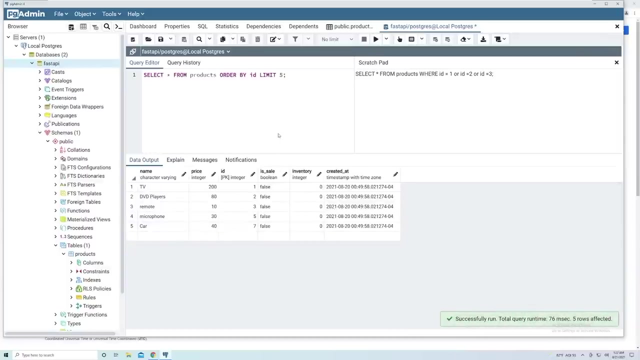 Okay, so that's expected. So let me add that back. So we'll say: I do an order by ID and then we'll limit it to five. So we have the first five. Now let's say that we want to skip a certain number of rows, because every time we search this we're going to get the same result. And let's say that we don't like the rest of the rows, that we actually did. 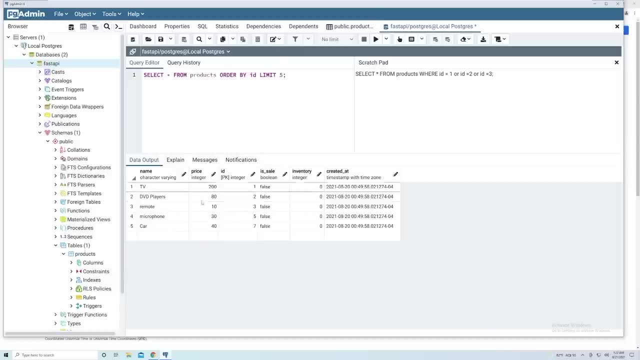 hint one Now, because you remembered we just відG whistle. Lets say we said a couple of times in the script: actually care about the first two results and I want to skip past them. we can provide an offset, So I'll do offset two, And so what that's going to do is it's going to skip past these two first. 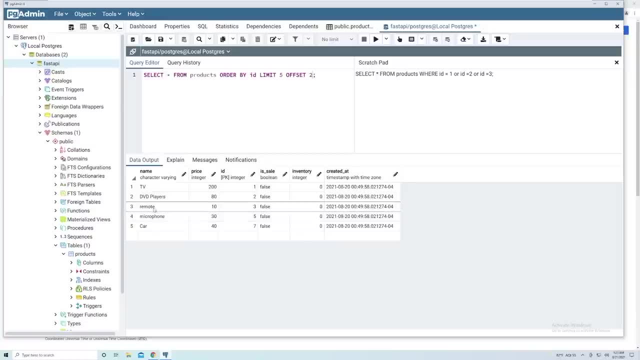 two results and then give us the next five. So we should see the first result be remote, then microphone, then car and then the two after that come after that. So if I search this, we could see that that first one is a remote and the last one is the pencil sharpener. 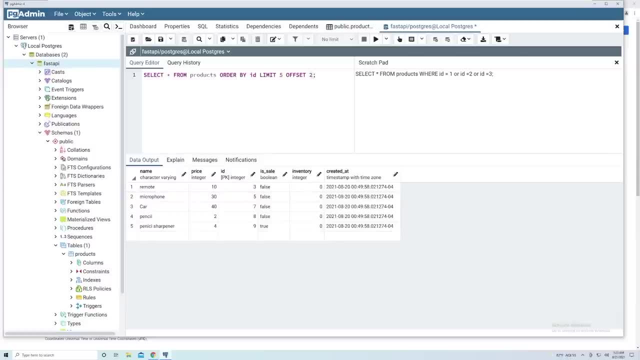 And then if I do an offset of um, you know five, it's going to skip the first original five. And so then we get pencil, pencil sharpener and keyboard. So you're going to see that you know, when it comes to limit and offset, these are going to come in handy When we start implementing. 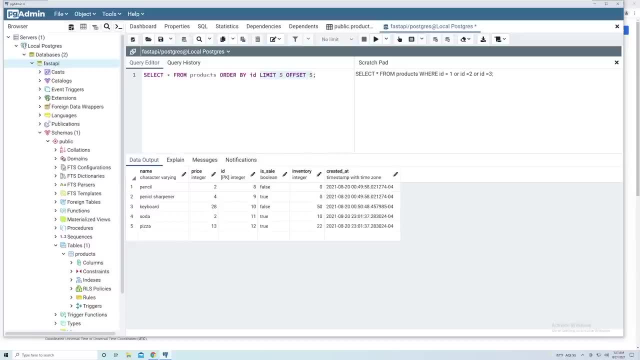 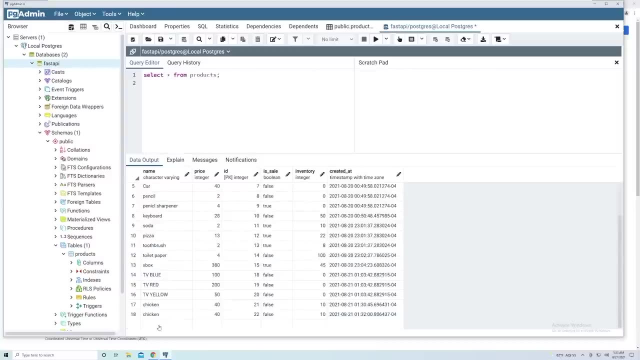 pagination. in our API we're going to definitely make use of the limit and offset keywords. Till now, we've been using PG admin to create new entries in our database by just going into the little gooey here and then just adding new values. 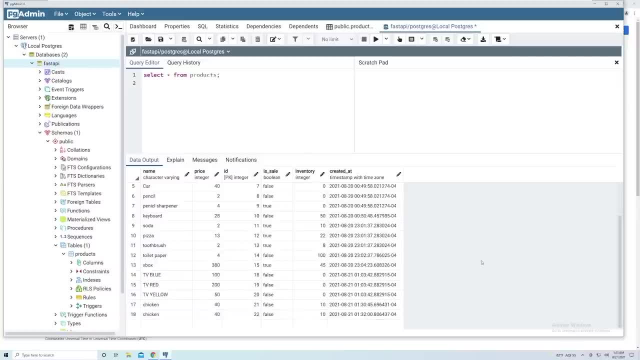 However, when you're actually working with the Postgres database, you're never actually going to do this. This is more for administrative purposes, but a real application is going to use SQL, just like we used to do with PostgreSQL. So we're going to use SQL just like we used to do. 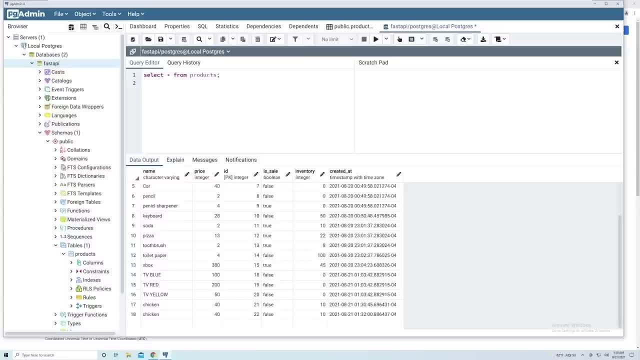 SQL, just like we used to do with PostgreSQL. So we're going to use SQL just like we used to do with SQL for making queries. we're going to use SQL for adding new entries. So let's take a look at what the command looks like for adding a brand new entry into our database. The command starts with: 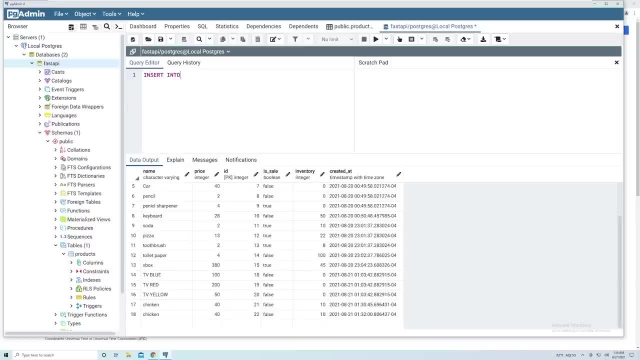 an insert, because we're going to insert a brand new row And then we say into, and then we're going to specify the table that we want to add a new entry to. Now in our database we only have one table, So it's going to be products, But here you would provide whatever table you'd like to add. 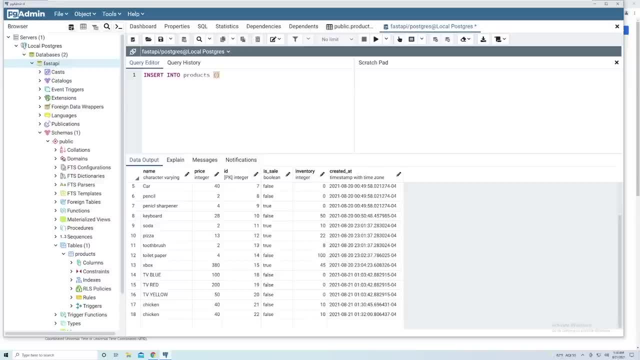 a new entry into, Then we have to do. what we have to do is provide a list of columns that we want to provide data for, And so I'm going to leave this blank for now. we're going to come back to that, And then we specify values, And then, here we're going to actually provide the values for each. 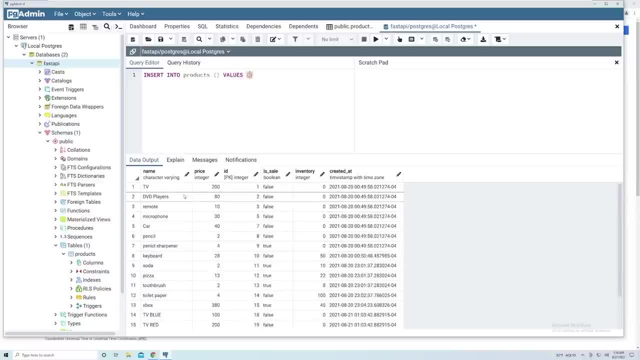 column, And so if we take a look at our products database, we know that the name is required, we know the price is required, And then that's about it. Alright, we can choose to provide an sale, but it's going to default to false, And then we can choose to provide an inventory if we want. 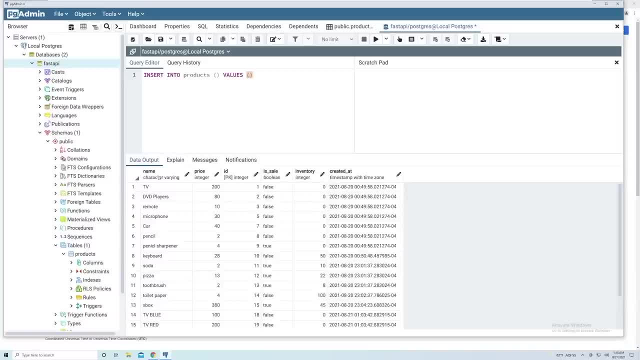 to. If we don't, though, it's going to default to zero, So we have to provide a name and a price, And it's ultimately up to us to decide what we want to pass in. So we know we need a name. 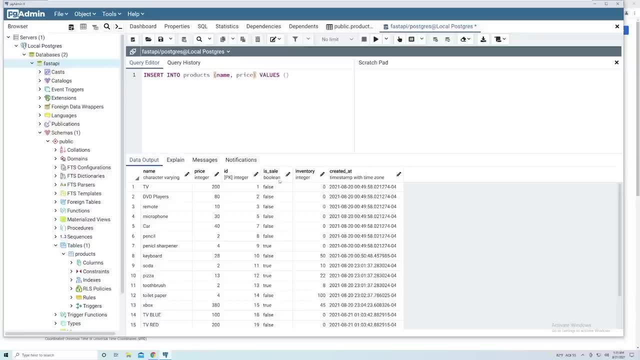 And we know we need a price. Now let's say we're going to let Postgres automatically give us. the default is sale value to be false. So we're going to leave that out because we're not going to pass in any data. So this column is just for all the columns we want to pass in data. 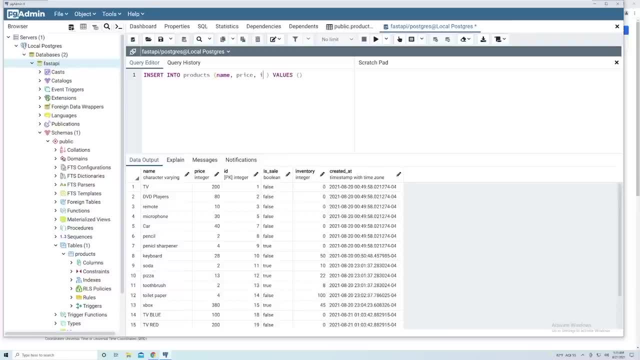 But let's say we want to give it a custom inventory value instead of just defaulting to zero. here we would provide inventory And then in the values column these are going to be the values that you want to actually provide for the name, the price and the inventory. 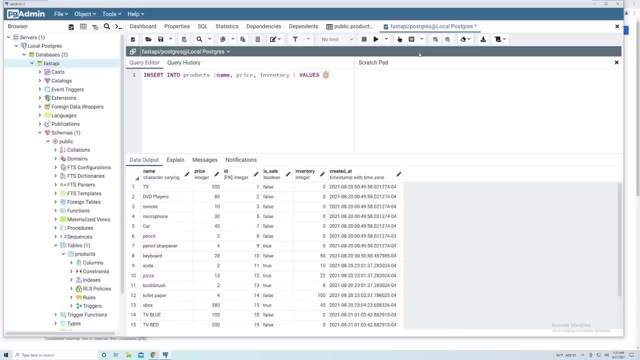 So let's go ahead and provide that. So let's create a brand new item, So let's give it a name, And the order in which you pass things has to match up with the order that we pass in here. So the first column that we're going to provide a value for is name, because it's the first one here. 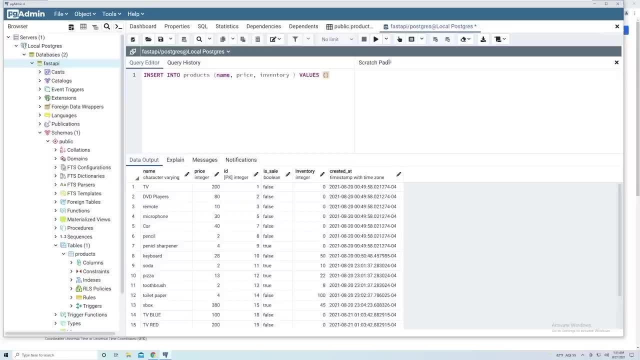 So what name should we give it And keep in mind? since it's text or varying character, we're going to have to put this in quotations And let's add in a tortilla. So now we're a grocery store, All right. 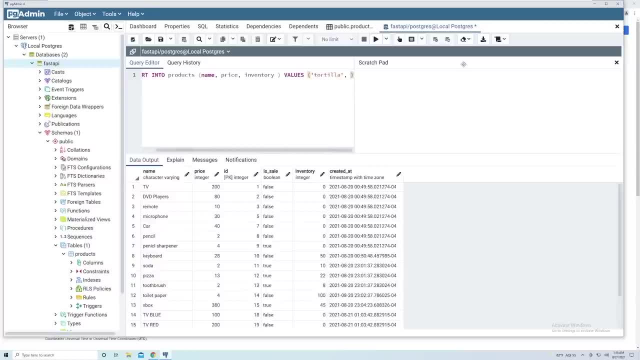 And then the next one is going to be a price. So how much is our tortilla going to cost? We'll say it's $4.. And then, finally, we have to provide an inventory value. So let's say we're going to have 1,000 tortillas. 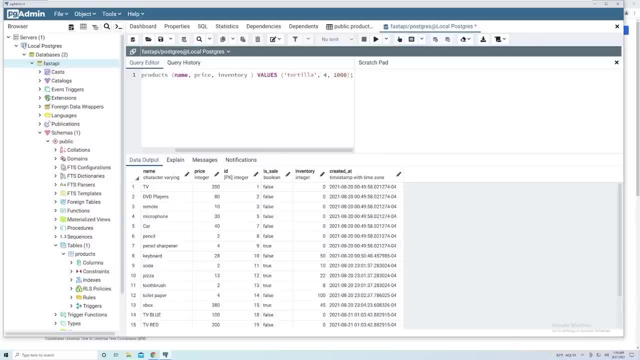 And then, as usual, you want a semicolon. All right, And so at this point, this is all we have to do to create a brand new entry. So let's hit, run And let's see what happens. So query returns successfully. 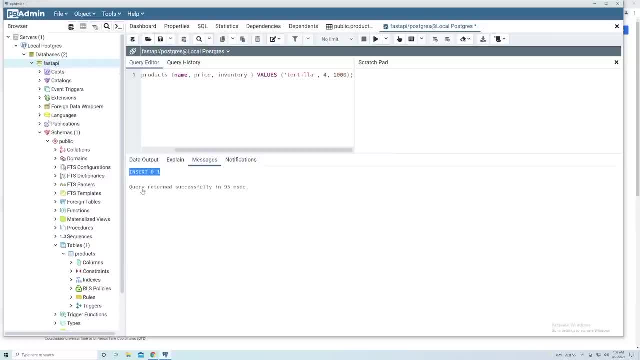 And so we see this insert 01.. And so at this point it says insert 01.. And then query returns successfully. So did we actually successfully insert something into our database? And, more importantly, what exactly does this mean? So if you see insert 01, that means everything worked perfectly. 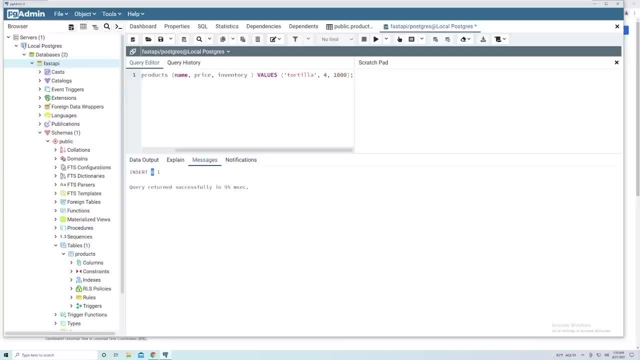 There was no errors. What this means is that first of all ignore the zero. So this means that we're using the default Postgres configuration. So this represents the OID, But I believe Postgres by default doesn't use that unless you specify it to. 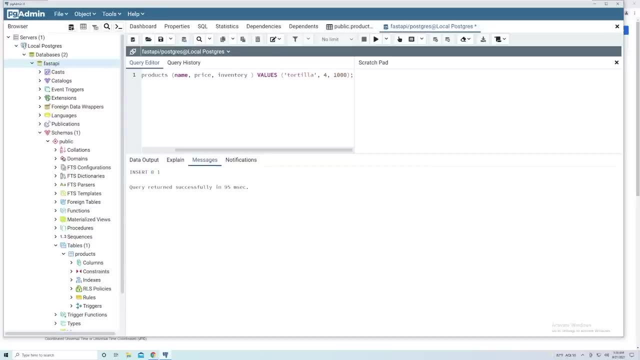 So it's going to give a value of zero And don't worry too much about that. That's kind of outside of the scope of this course. We're not going to mess with that, But instead what we want to focus on is that second column. 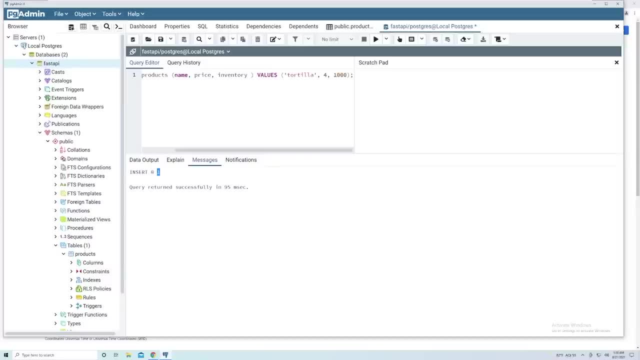 So this means that we inserted one row, So that means our insert worked perfectly. So let's take this, And what we're going to do is, first of all, I'm going to copy this, Cut it out, Actually paste it into my scratch pad for now. 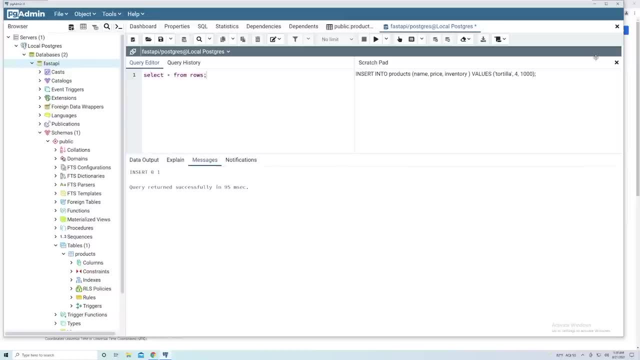 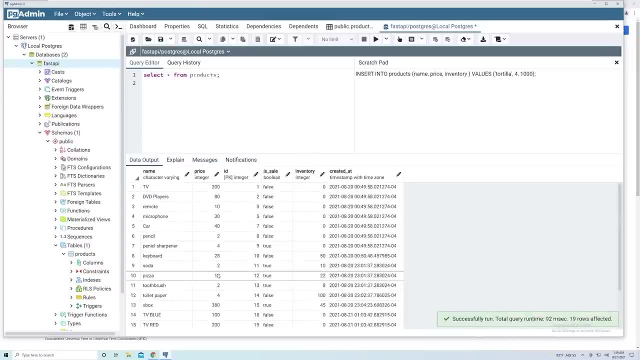 And then we're going to say, select star from rows, Sorry, select star from products, And we're going to run that. And so if we go to our bottom, we should see our brand new tortilla, And so we provided the tortilla value. 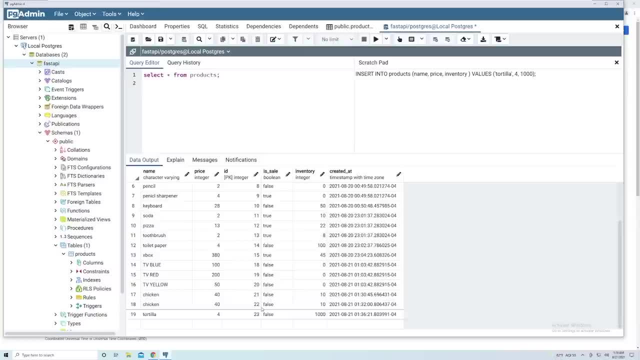 We provided the product, We provided the price And we did not provide an is sale, So a default is false. And then we provided an inventory. Now, if I copy this again and paste it back into here And if I move the name column right after the price, 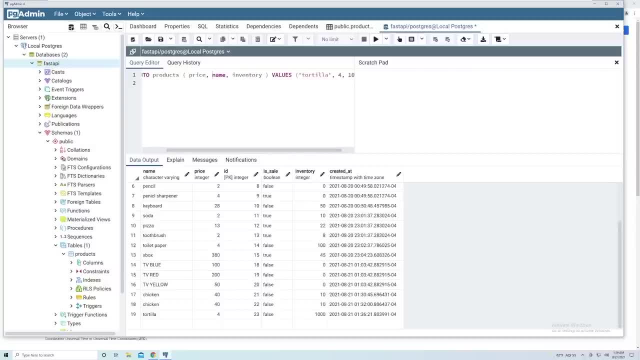 Well, now SQL is expecting me to provide the value for price first, then name, then inventory. So then I would have to take the price, move that over To the first column and then move that. move that into the first entry. 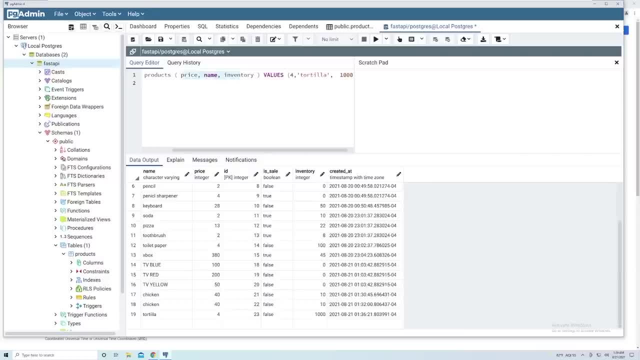 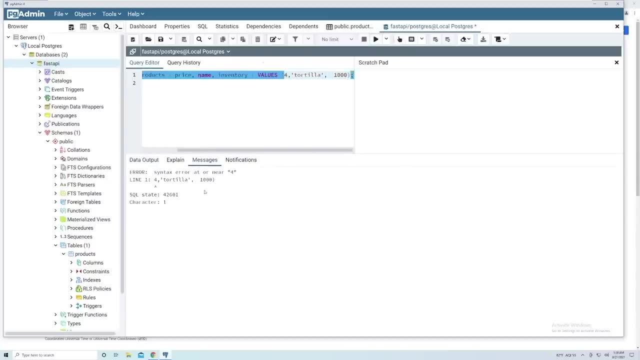 And then we have the name and then the inventory, And so, keep in mind, the order here has to match the order here. So once again, I'm going to go ahead and just add this again, because, why not? And so now, oops, it looks like we have an error. 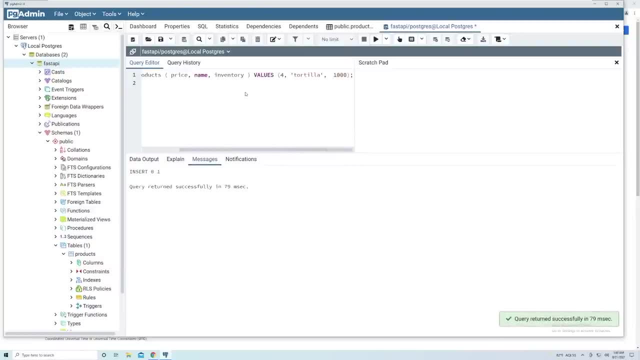 What happened here? All right, there we go. I guess we just needed that space, And so now it's in there, and you'll notice that once again we get the zero one, So that means everything was inserted properly. So now we should have two items in our database with the name of tortillas. 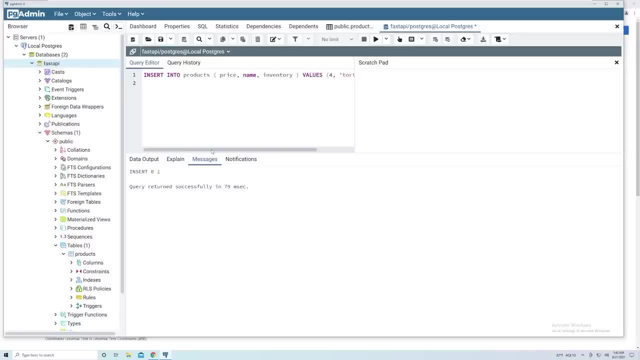 And when you're working with With Postgres, and especially with an API where we want to create a new post, like in our application. the general convention in an API is, once we create the new post, we want to return that data back to whoever sent that request to the API. 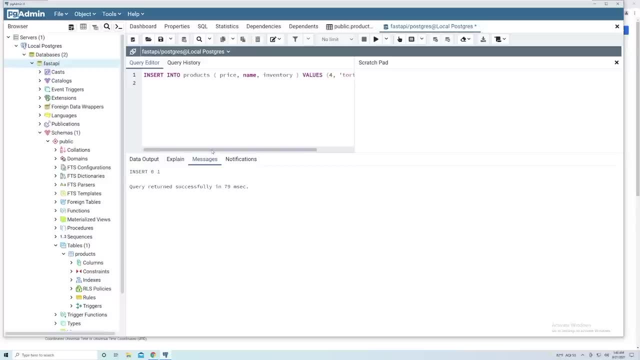 So we want to get that brand new, brand newly created post with the new fields, like the created ad field and all the default values, and send it back to the client or the front end. So how do we get Postgres to automatically return it, Because right now it doesn't seem to do that? 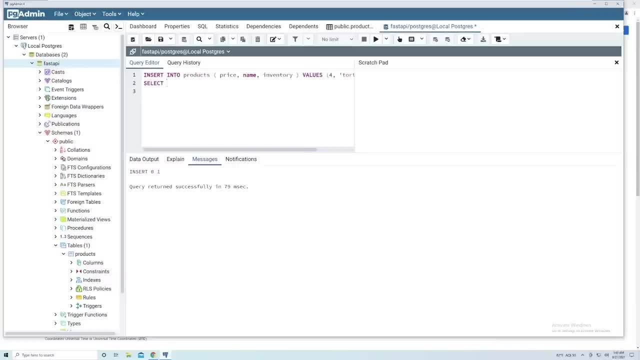 And we could, you know, just provide two statements. right, I can add in a second statement that says select star, you know, from products. This is going to dump everything we could potentially. you know filter on. you know where name equals, you know tortilla or something like that. 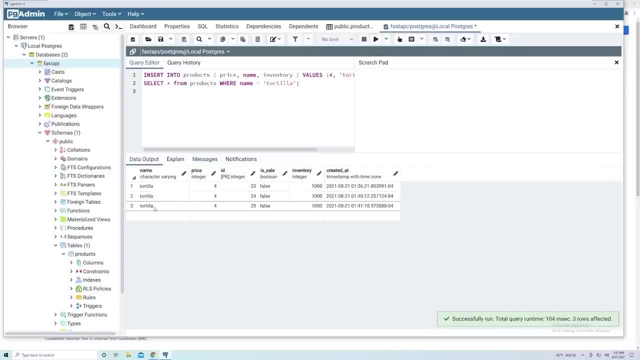 And then at that point we should have three entries. But that's one way of getting back the result. However, there's a much easier way within Postgres. So, first of all, I'm going to change the name, I'm going to add a new item and say: this is a car and I'm going to give it a price of 10,000. 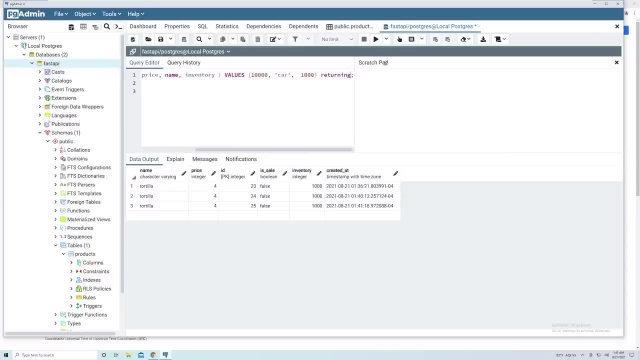 And what we can do is we can pass in a keyword called returning, But this is going to return the newly created item or items, if you want to insert more than one item, And then here we have to specify the columns that we want for the newly returned items. 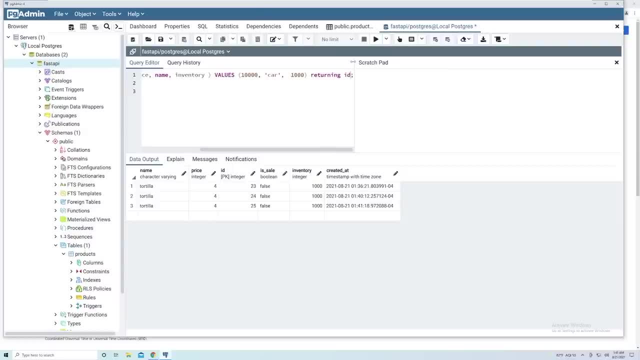 So if I do star, that's going to return every single column. If I do ID, this is just going to give me the ID of the brand new created item. I'm going to return every single column. So if I try this now, look at that so it creates the new entry we can see that has an ID of 26.. 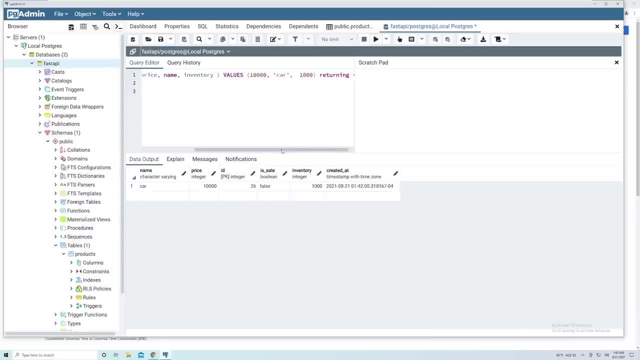 And it gives back the entire row. Now, if you want to insert more than one row at a time, what we can do is we just do a comma here after values and then just provide the data for the next row. So we'll do. we'll create a new item. that had cost $50.. 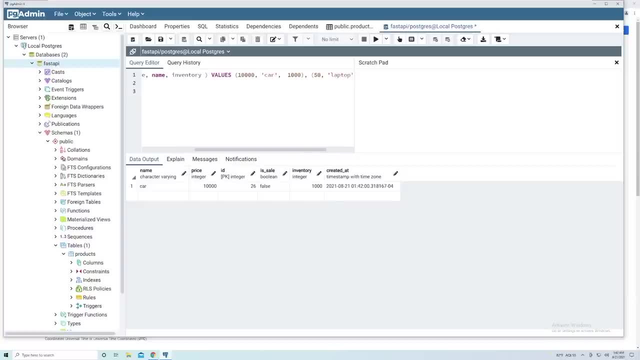 And this is going to be a laptop, And then we'll say there's going to be an inventory of 25 of them, And then if we wanted to add another one, and we could just do another comma and then add some more values in. 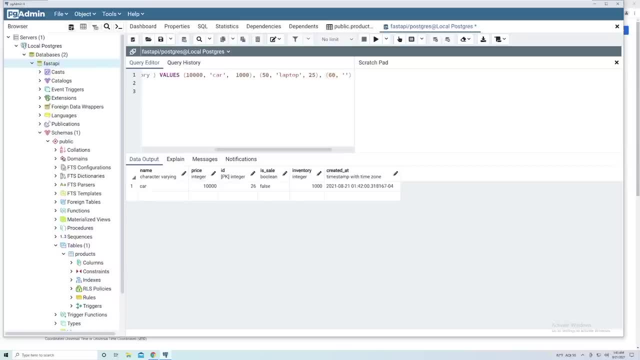 So we'll give this a price of 60.. This is going to be a monitor, And then we'll say we have four of those, And so here we can go ahead and run. You can see that it added three items And then it returned all three, because we have the returning keyword. 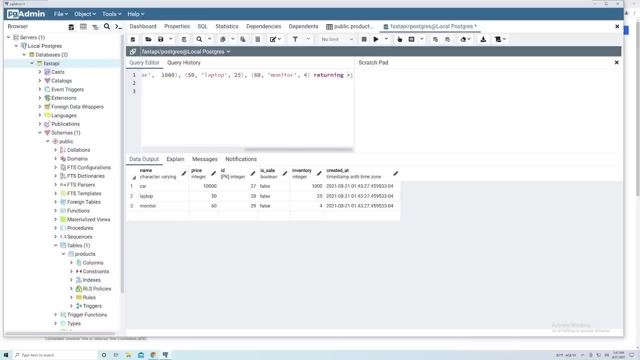 And if you wanted to, we could just say: I want the ID. we can just say I want the ID and the created at field, Maybe the name as well. I run this. we can see created another three new items and then return just those three fields. 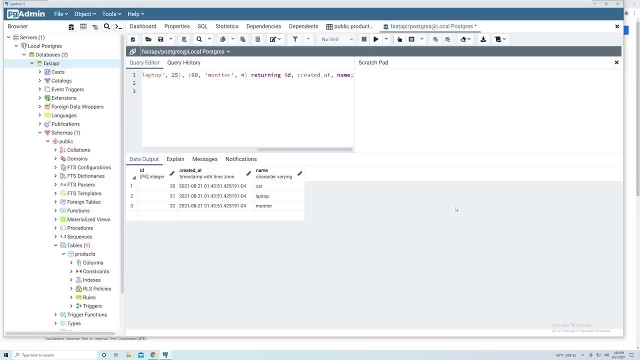 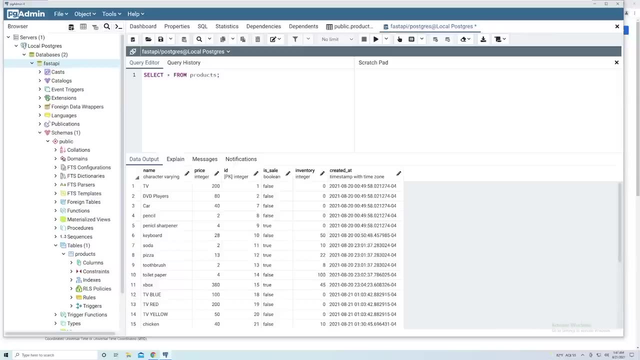 And so that's pretty much all I wanted to cover. when it comes to creating new entries in the database and inserting new rows into a table, Alright, so in the last lesson, we learned how to insert new entries into a database. Let's now figure out how to delete entries. 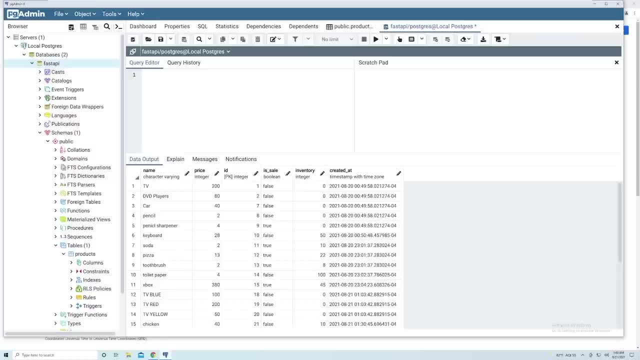 So let's clear out this query real quick. And the command to delete a entry from a database is going to be delete. who would have thought, right, delete? then you say from, and then you provide the table that you want to delete a row from. 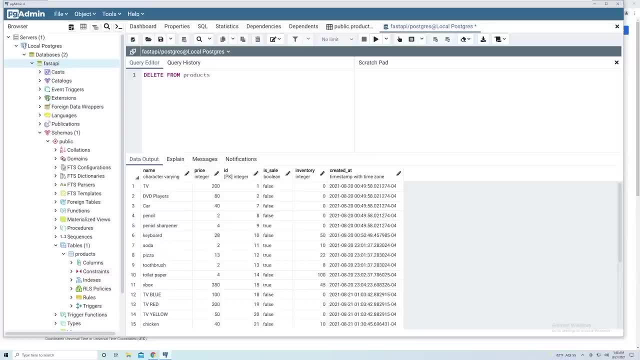 So we'll say products, And then we want to specify conditions. So what is our match criteria? What rows do we actually want to delete? we have to tell SQL: I want you to delete this specific, specific row. So what do we usually match on? 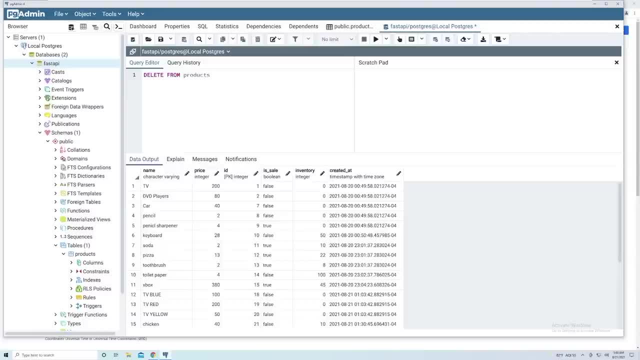 Well, if you take a look at our API- our, specifically our- delete endpoint, the user provides the ID of the product they'd like to delete, or I guess in our application it would be the ID of the post we'd like to delete. but we're working with products. 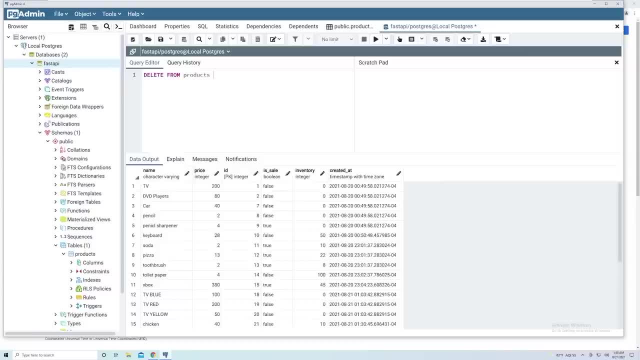 So we'll say: you know, just like with a regular select query, you say where we can say ID equals and then the ID of the product we want to delete. So let's take a look at one of these products. I'll grab a product 10.. 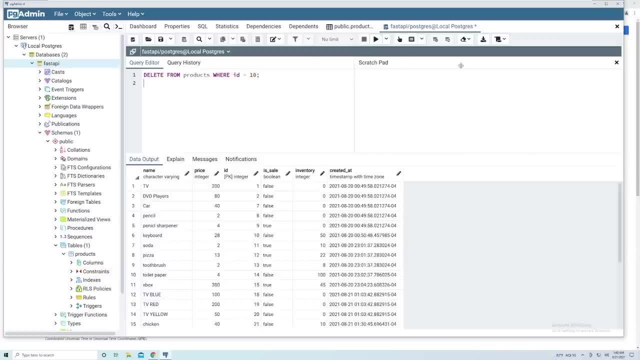 And then let's run this And then afterwards let's actually do a select star from products So we can see all of the products afterwards just to verify that the ID of 10 or the product with an ID of 10 got deleted. 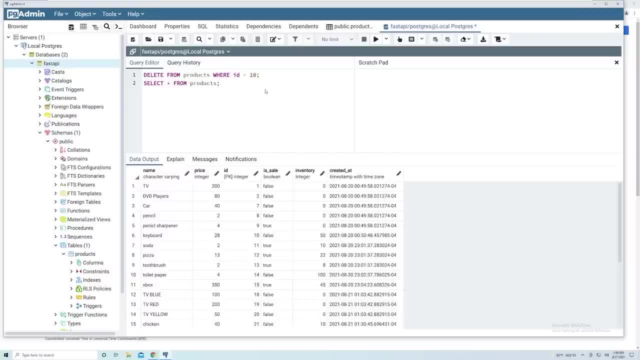 So you can pass in as many SQL commands as you want here. So we'll run that, And so it ran, And then we can see that we, the product with an ID of 10, was deleted. Now I'm going to change this to 11.. 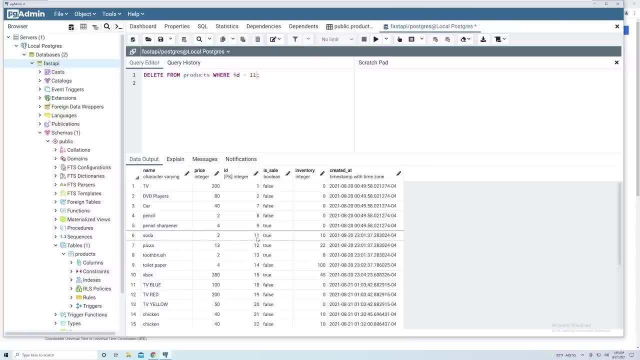 Because there's no longer a product with an ID of 10.. So I'm going to delete this product. But what we can do is we can tell Postgres to actually give us back the specific entry before is deleted. So we can see what that looked like. 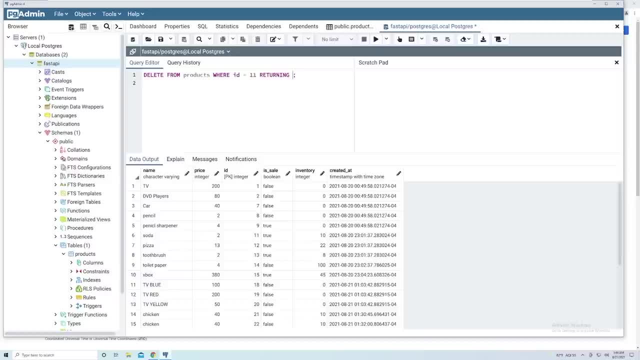 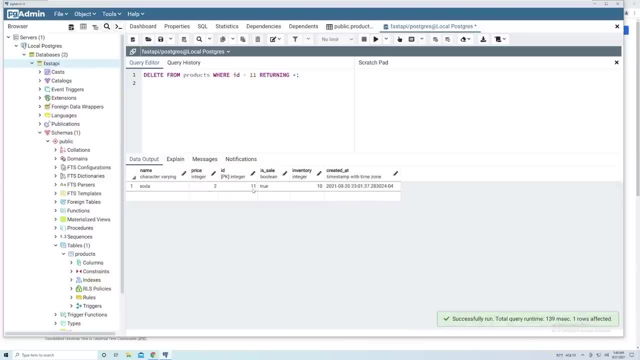 So we could just pass in the returning keyword, just like we used with the insert statement, and then we specify the columns we want. So I'm going to say all of the columns And then if we run this, we can see that it deleted the product with an ID of 11.. 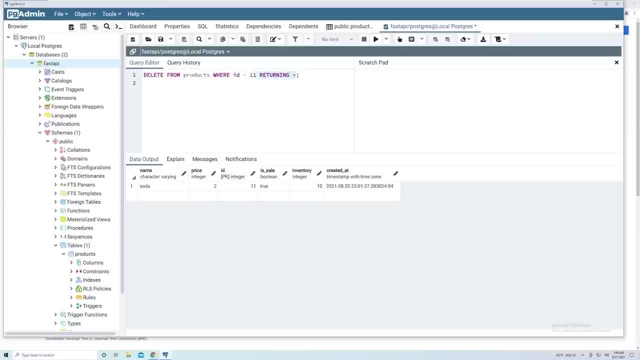 And we can see what that product looked like And keep in mind. if I don't pass any of this data and I just run this right, you'll see that it says a delete of one. So this is just telling you how many total rows are deleted. 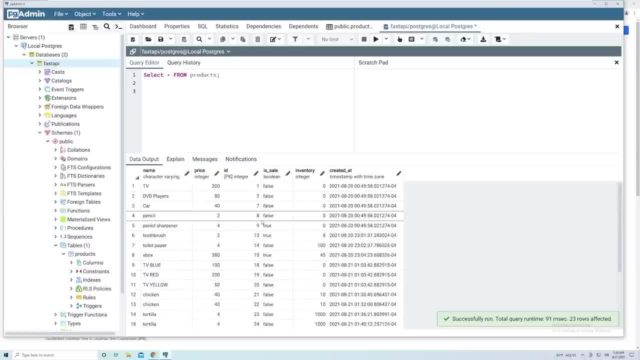 Now let's say that we want to delete multiple products based off of a criteria. So let's say we want to delete any product that has an inventory of zero. how do you do that? Same exact command we just have to match on any product with an inventory of zero. 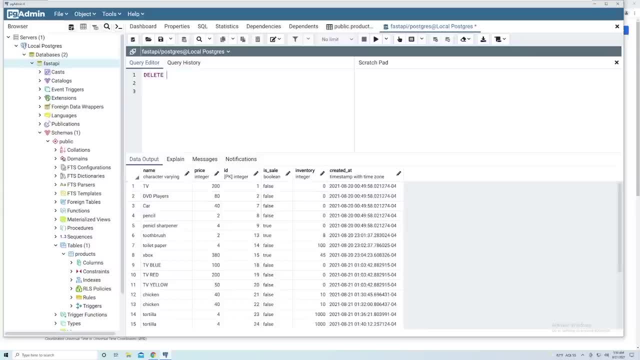 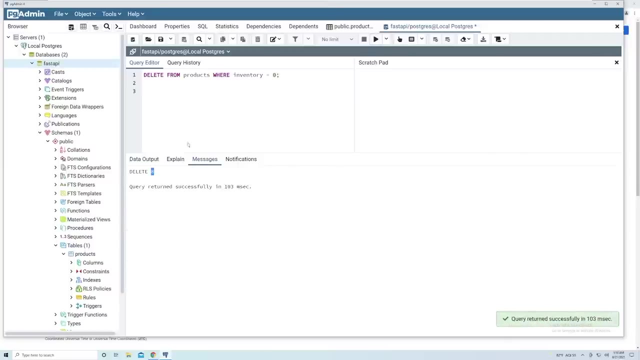 So let's say: delete from products, table where. and then we'll just say inventory equals zero. So this should work. We should delete every single product with an inventory of zero. We run this. we can see it deleted eight rows. Let's just do a select star from products. 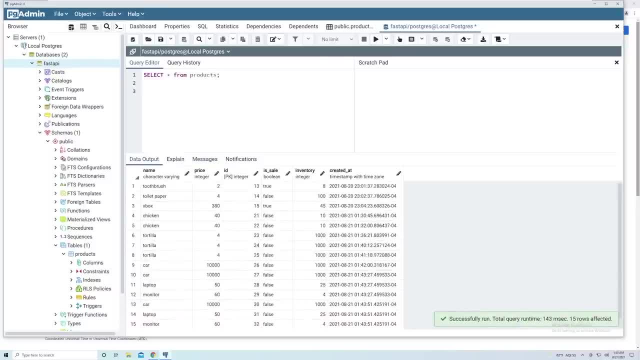 And you can see we no longer have any products with an inventory of zero. Alright, so we saw how we can insert new data into our table And we saw how we can delete entries from our table. I think the next logical step is to figure out how to update a pre existing row. 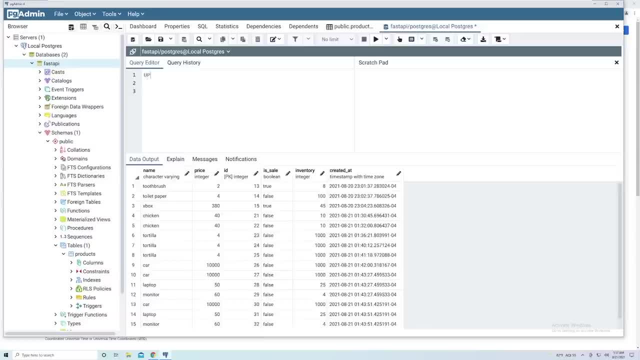 So the command for updating is going to be, as you guessed, update, And then we have to specify the table that we would like to update, And so in this case, it's going to be the products table, And there's gonna be two things that we have to pass in. 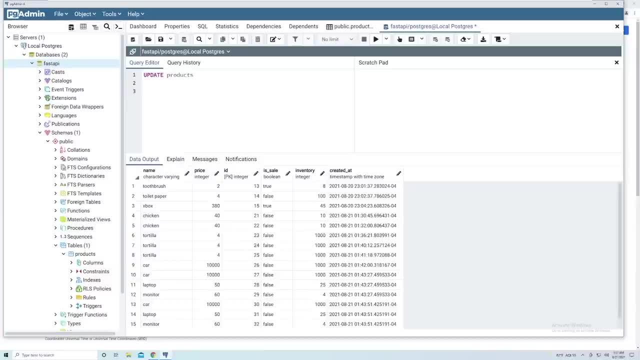 So, first of all, we need to specify which entry we want to update. we can update more than one entry at a time, But you know, just like when it comes to deleting, if you take a look at our API that we've built so far, the user provides the ID of the specific post they want to update. 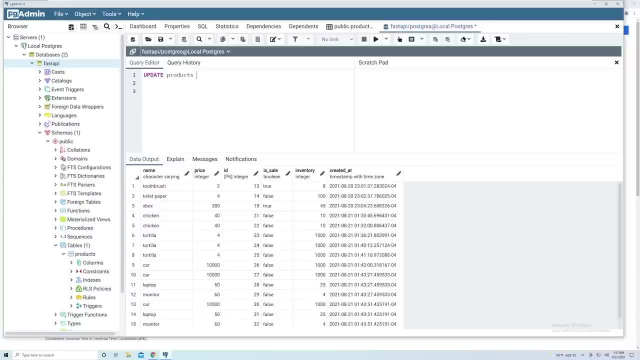 So normally we're going to update based off of the ID column. So we'll say where you know, just like the select statement or the delete statement, we can say where ID equals and then the specific product of the ID and the specific ID of the product that we want to delete. 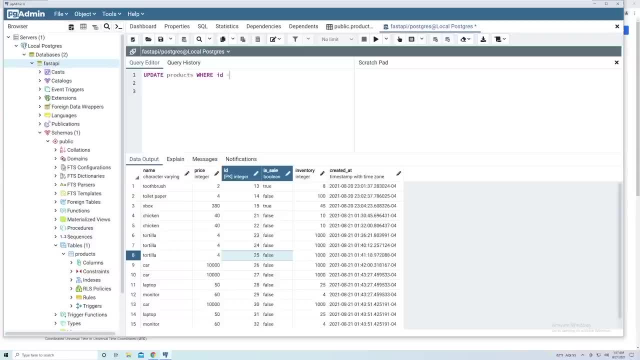 So let's say we want to delete one of the tortillas, So an ID of 25, sorry, not delete but update. So we'll say 25.. Then we want to pass in all the columns that we want to update. 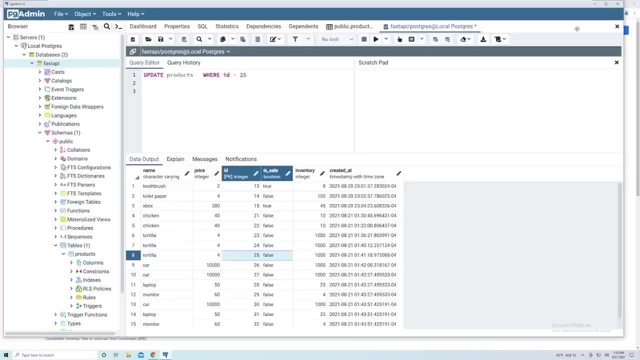 So we pass in the name of the column and then what the new field should be. So let's say a name column. I want to rename this to be a flour tortilla. And then let's say: I also want to update the price. 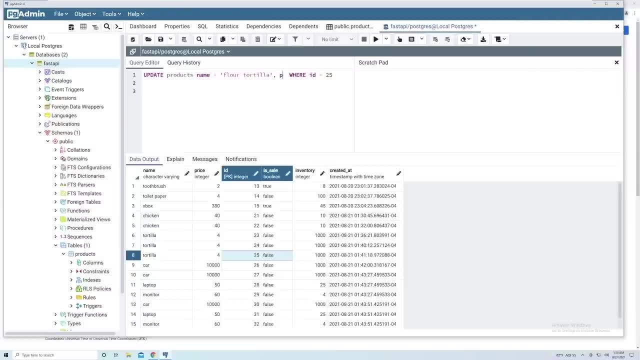 So I could say the price equals and then 40. So right now the price is four and the name of tortilla. it's going to now be flour tortilla and 40. I run this and don't forget the semi colon at the end. 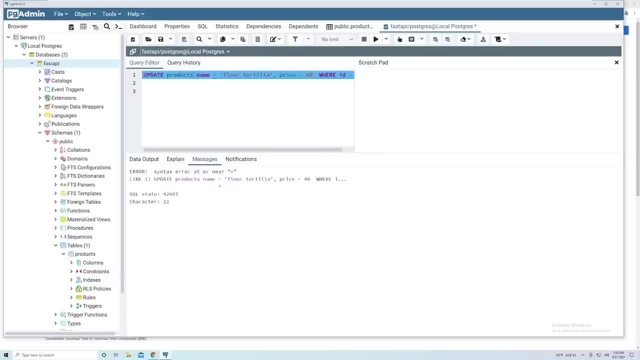 And I realized I forgot one key word. So before you pass in all of the new values, we have to use the keyword set. So it's update products. then we want to set these columns. then I run this and we can see that we updated one field. 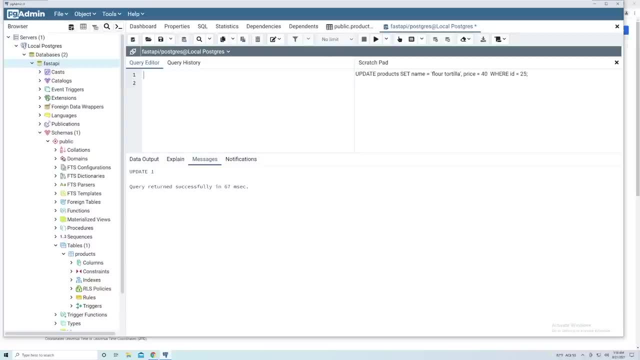 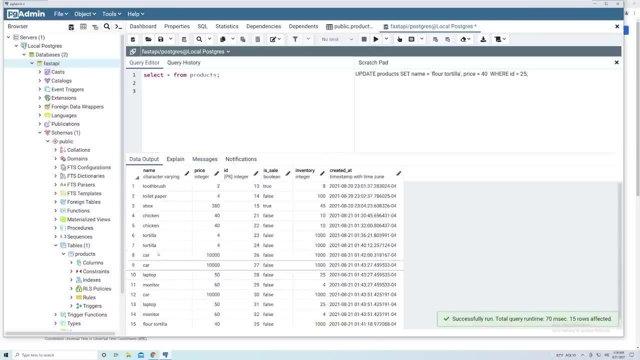 And I'm going to copy this, put it in my scratch pad for now and just do a select star from products. And so if we take a look at our tortilla- so now it's called flour tortilla- we can see the ID is still the same because we didn't change that. 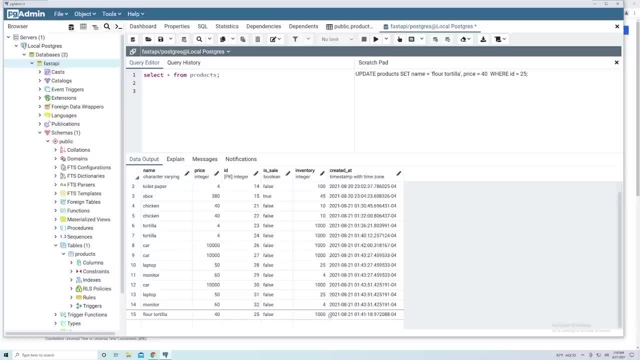 And the last one, The price got changed. However, all the other fields have all remained the same, So that's good, But, just like when it comes to inserting new data, we generally want to return the newly updated product to the user. 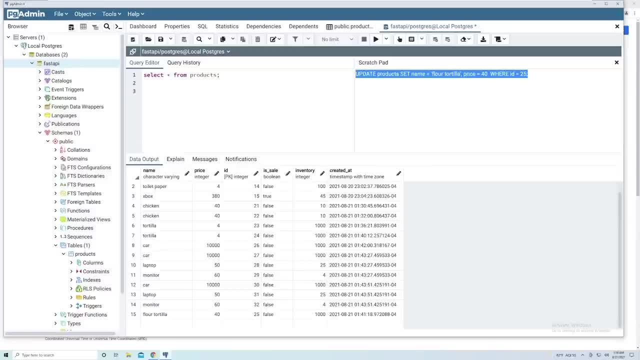 So how do we do that? we could just use a returning keyword. I'm going to copy this again And let's update a different product. So I'm going to update the car, which is a ID of 30. And let's just say I want to update one field. 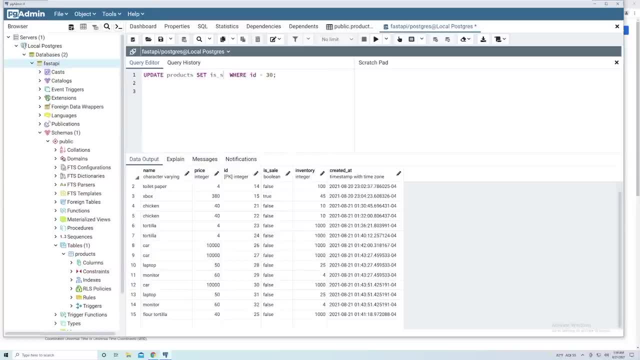 Also. I'll remove all these And I'll just Say I'm going to update the is underscore sale field to be to set it to true, because right now it's set to false. We'll set that to true And then we can say returning star. 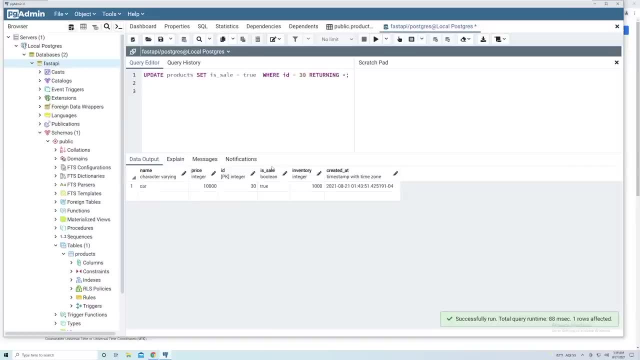 If we update this, we can see that we now got the car, we can see that the is sale set to true and it returned that data and it was successfully able to update that. Now let's say we want to update multiple rows. 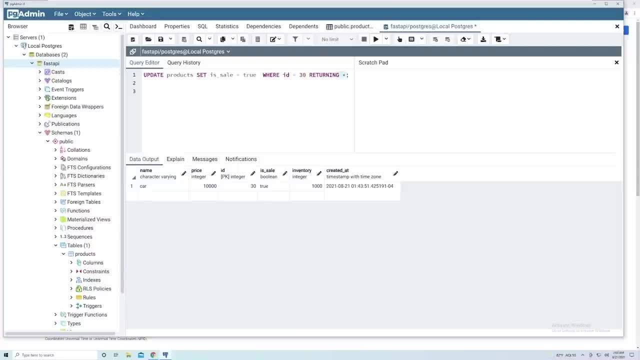 And let's say I want to update, we'll just let's just update everything, right? So if I don't pass in a specific condition, I can update every column, or I can specify a condition and then update just those columns. 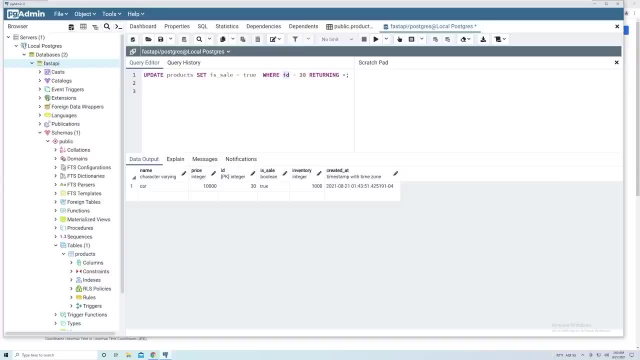 So let's, let's say I want to match any, any product with an ID of 15 or greater, so an ID of greater than 15.. And I want to set the is sale to be true. If I run this, we can see all of the. 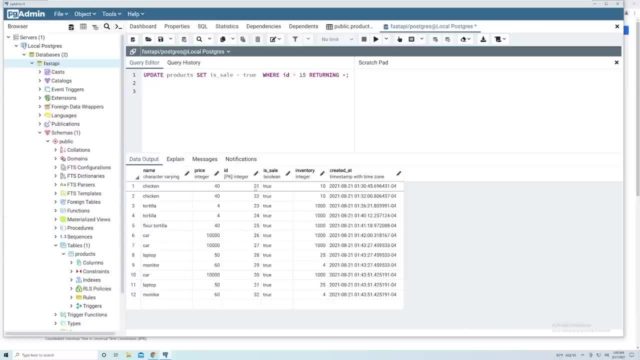 Entries that it was that it updated. So now all of these entries- which all have an ID of greater than 15, have all, all have the is sale column set to true, And so that's how we update entries within a Postgres database. 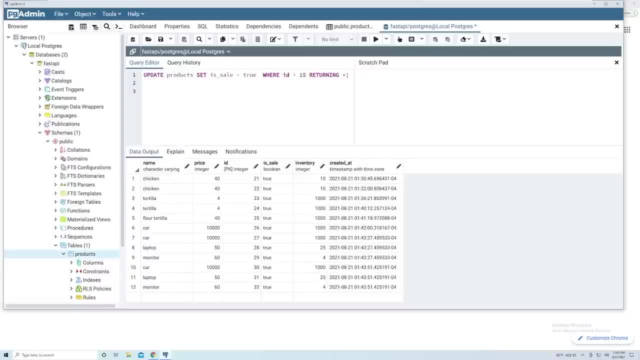 At this point, I think we have a good enough foundation when it comes to working with Postgres. We're able to successfully query a database, insert new rows, delete rows and update rows. So I think it's time we finally started to go back to our code and figure out how we can actually work with a database within. 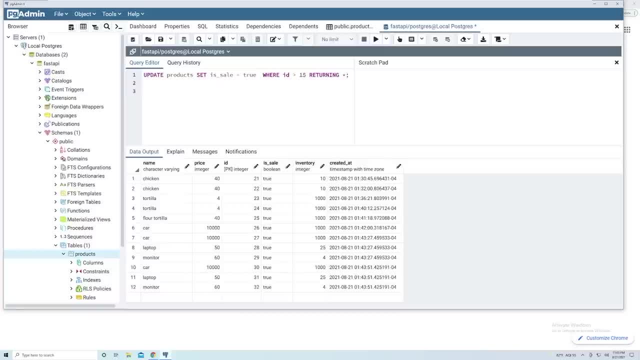 a Python or a fast API application. But before we do that, I want to do a little bit of cleanup So with our database we no longer need our products table. So what you can do is you can go ahead and delete it, So you can just right click and then hit delete or drop Technically, if you don't want. 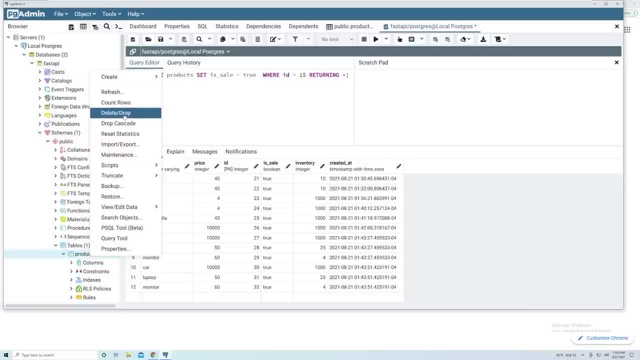 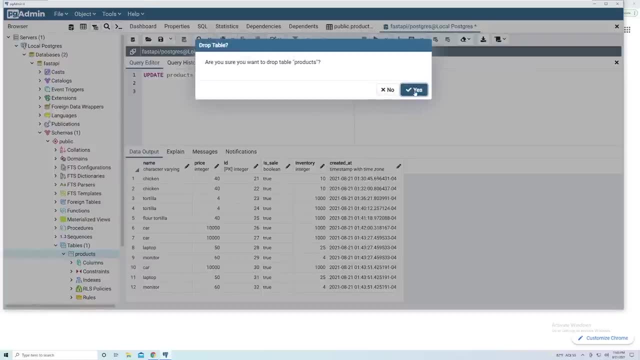 to delete this and you want to keep it for now, just for reference. you don't have to delete your table. it's not going to impact anything else, So you can keep it, But I'm going to go ahead and delete it because we don't actually need it anymore. We'll just do that: hit yes And then. 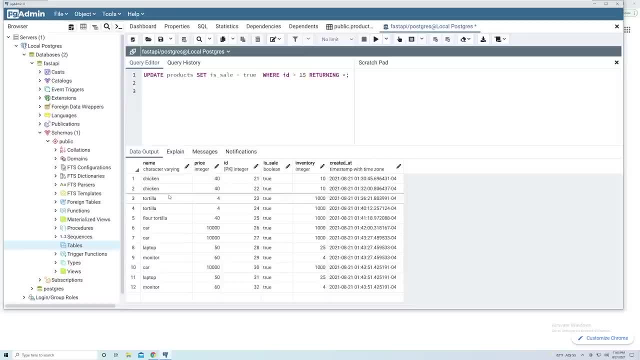 it's going to delete that and we should no longer have tables And I'm also going to move over to another machine. So when we go to the other machine you will see a whole bunch of other databases. But those are all databases for my other project. make sure you just focus on the. 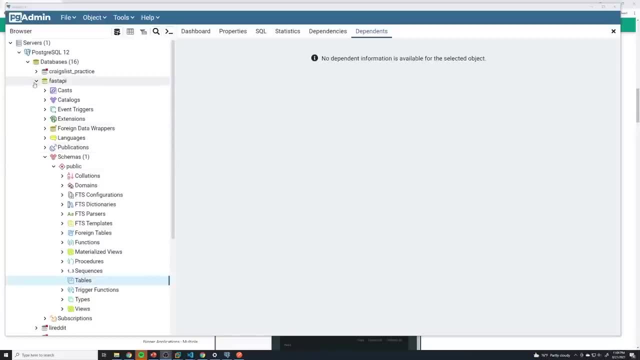 fast API database. Alright, I'm back over to my new machine. you'll see that if I take a look at my database, there's going to be a whole bunch of other databases, But I've got my main fast API database, So that's what we're going to be working on. Don't look at any of these other ones And 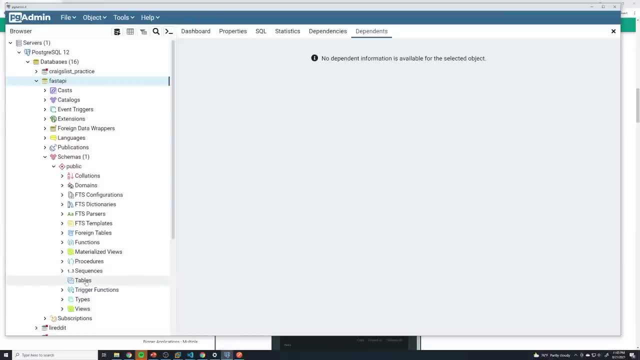 within here it's going to be pretty much empty. I've got no tables, And so we're going to go ahead and create our table for our social media application. So you know, we've been working with posts, So I think it makes sense to create a table for posts, And before we do that, we have to figure out: 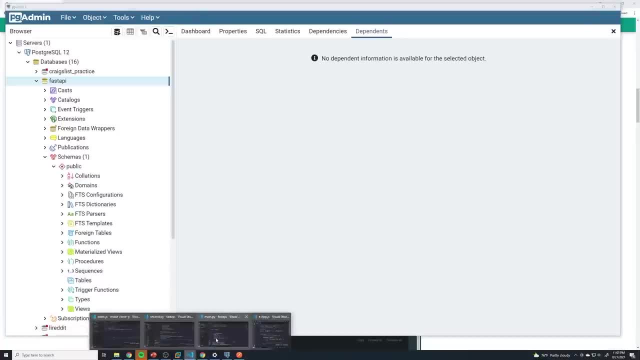 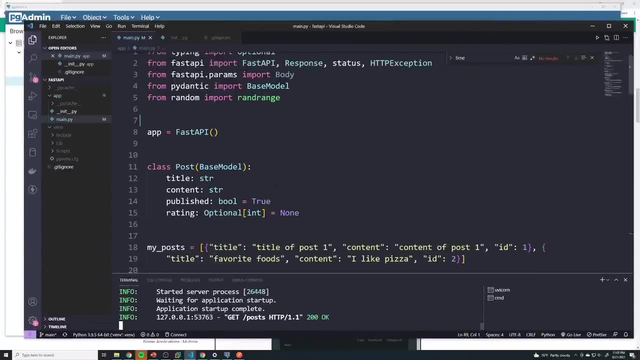 exactly what are the columns for our specific table. And to do that, I think best to actually take a look at what our application looks like at the moment. And so if we actually take a look at a structure of a post, we know that it's going to have a title, we know it's going to have a 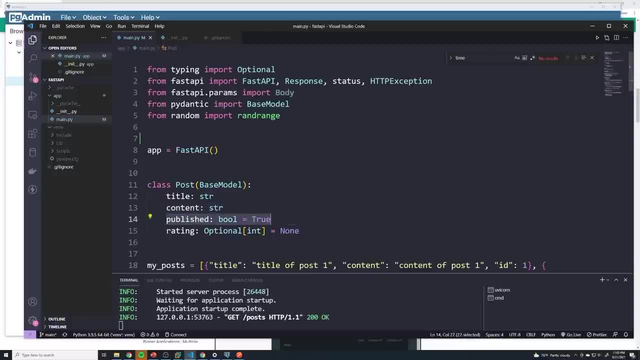 content we're going to. we know it should have a attribute called publish to determine if it's going to be a post, And we're going to get rid of this rating. that was just for demonstration purposes, So I'm going to remove that for now. So it should have a title content published And like: 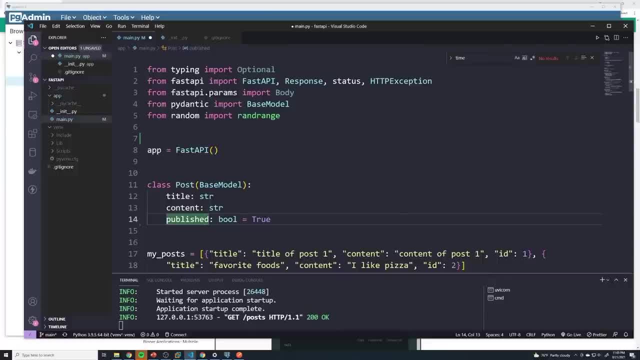 any other item. when it comes to a database, we're going to have an ID column as well so that we can- we can- uniquely identify each entry. And then we're also going to have a created ad field to see, to track when the specific post was added to the database. So we've got essentially five columns. 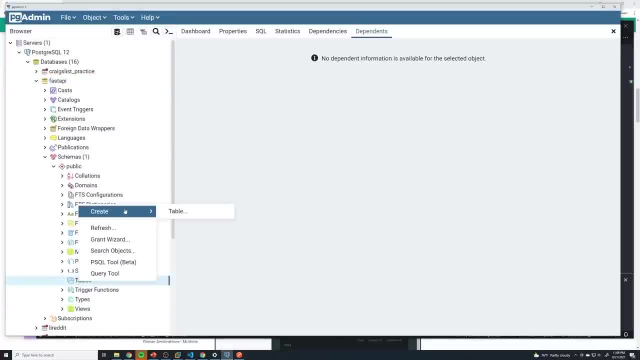 And then, once we have that, we can go ahead and just do what we did before. We can go to tables. we can hit create table- This table posts because it represents our social media posts. And then we'll go to the column section and start defining our columns. The first one is going to be our ID column And so, with our ID, we 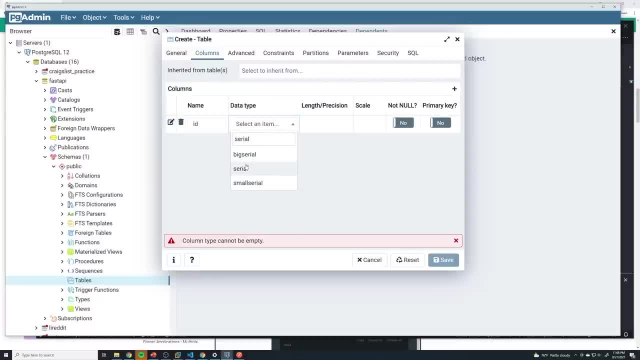 want to do serial. So this is going to cause it to be an integer that automatically increments for us, And then that's going to be our primary key, as it was before. We'll add another column for title. This is going to be a varying character, or character varying, not. 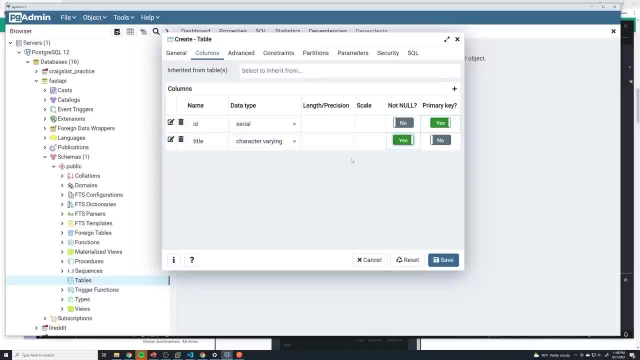 null. it's going to be set to true. we can't, we don't want to be able to create a post with a, without a title. Then we're gonna have a column called content. I believe that's what we called it here: Content- Yep, Once again this is going to be character varying And once again, this is going to be. 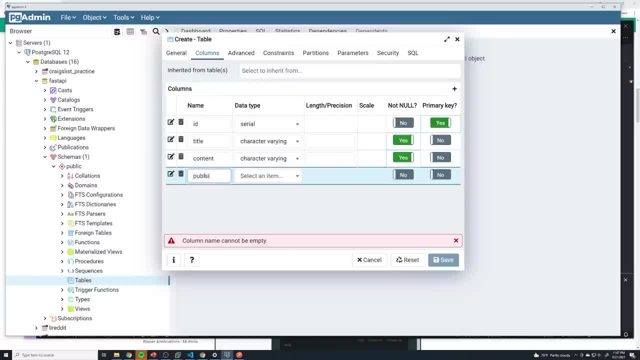 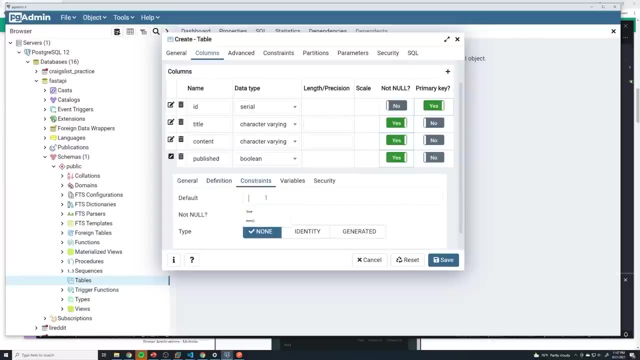 not null. Then we're going to have a published column And this is going to be a Boolean. This is also going to be not null. However, I'm going to provide a default value. So if I do leave it blank, it's going to default to true. 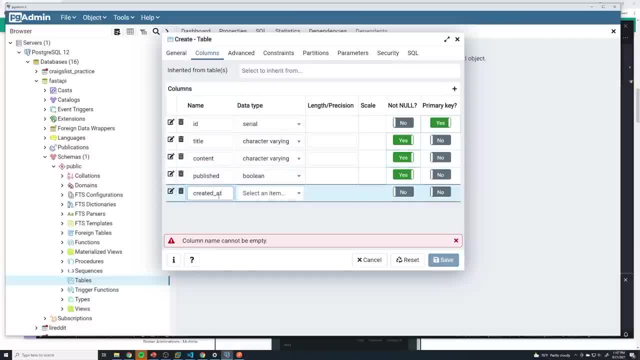 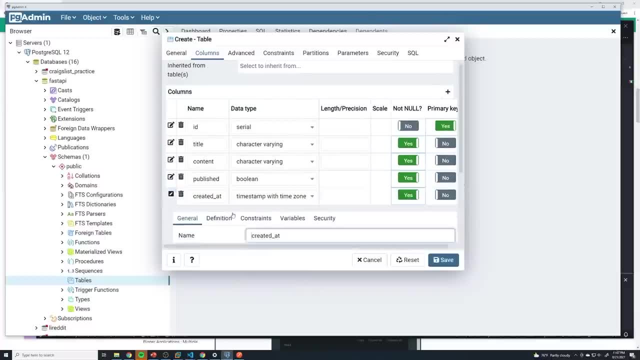 And then, finally, we're going to create the created column, And this is going to be a timestamp with timezone- This is also going to be not null- And then, just like we did before with our products, we're going to add a constraint, But that is going to be now, so it's going to grab the current time. 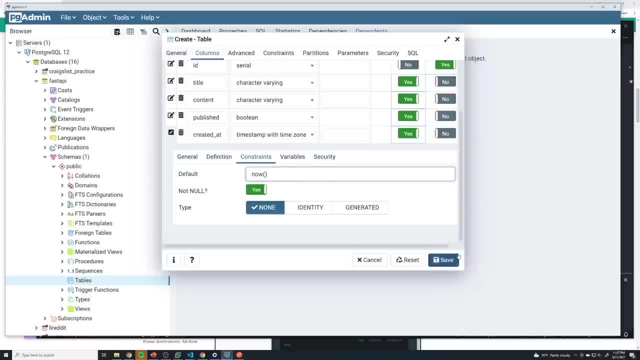 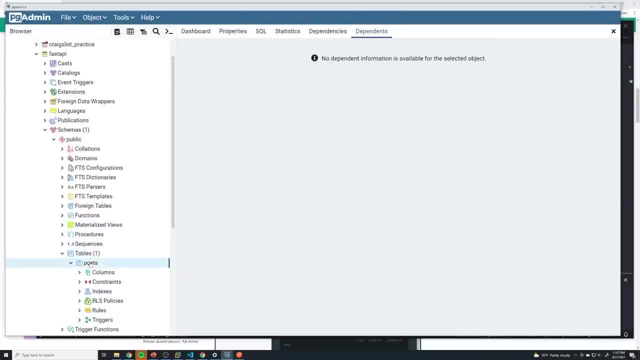 whenever we add this entry and it's going to automatically add it to that column, And so at this point we've got our tables defined. we can go ahead and hit save. If we right click on posts and then go to view and edit data, we should have essentially what is an empty database, And for now we know how to. 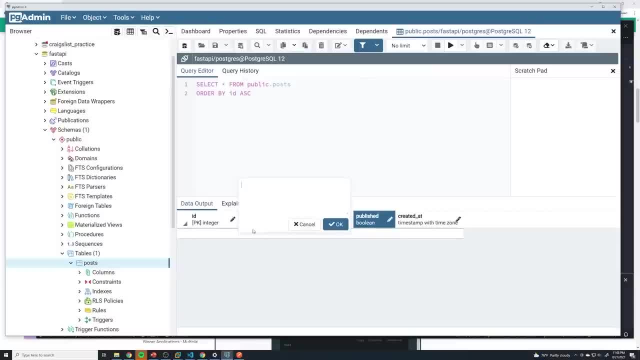 insert data. we can do it either through SQL or we can just do it to here. I'm just going to do it through here, just because it's a little bit quicker for now. So I'm just gonna say this is my first post And the content is: we'll say: 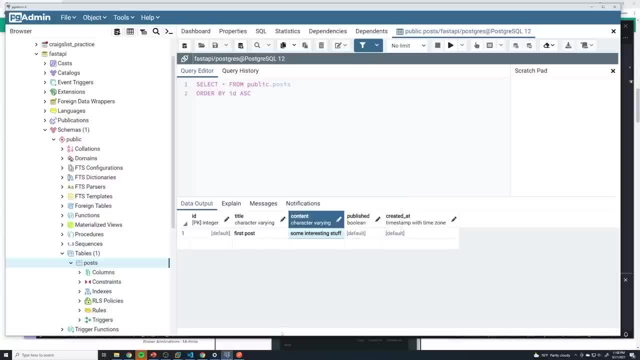 interesting stuff. But you go ahead and just create a couple of posts And then I'm gonna add my second post, Right, and then we can just hit save, And so now we have two posts in our database, So we can start working with that. 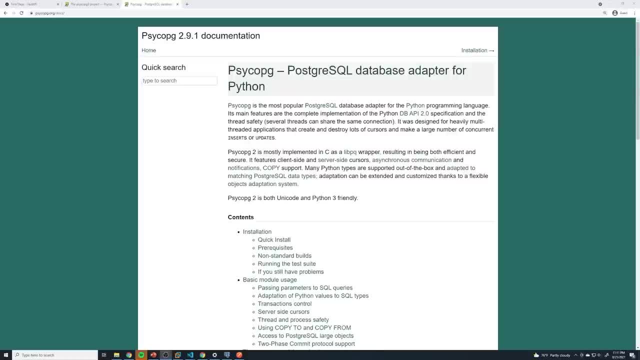 When it comes to working with a Postgres database within a Python application, we're going to need a Postgres driver, And so there's going to be a couple of different libraries that are going to do that. that can do that. we're going to use this library. 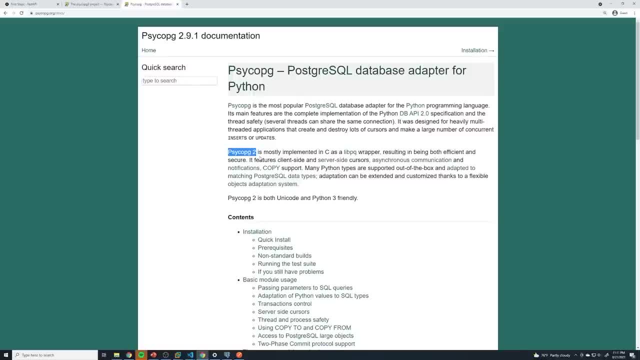 right here And I believe in a couple of months a version three is coming up, But right now this is the latest version, So head on over to the documentation and it's going to show you how to just quickly set this up. 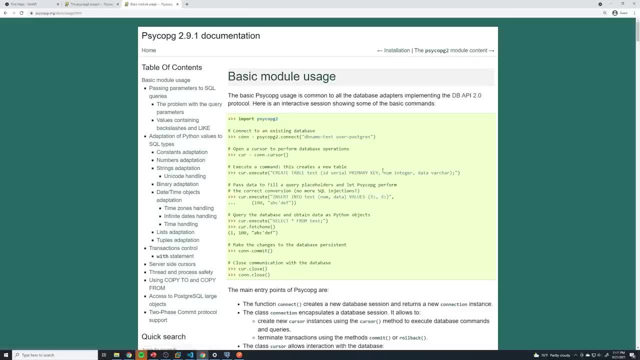 And so if we go to basic module usage, this shows us how to set up a connection to our database, And so we're going to import the library And then we're going to set up a connection, And hopefully this is big enough for you guys. So you just say connection. 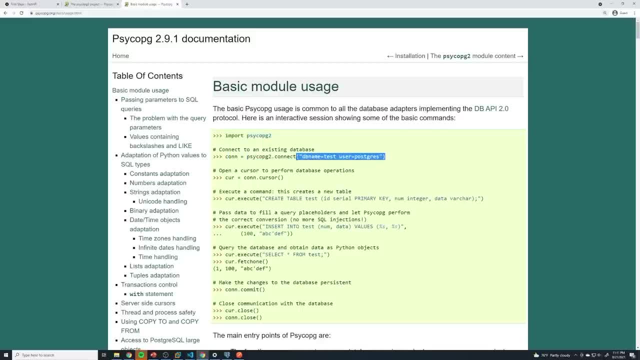 And then here we pass in all of the data for our Postgres instance. So you know what's the IP address of the Postgres database, What's the Postgres database that we want to connect to, what's the port number, things like that. And then 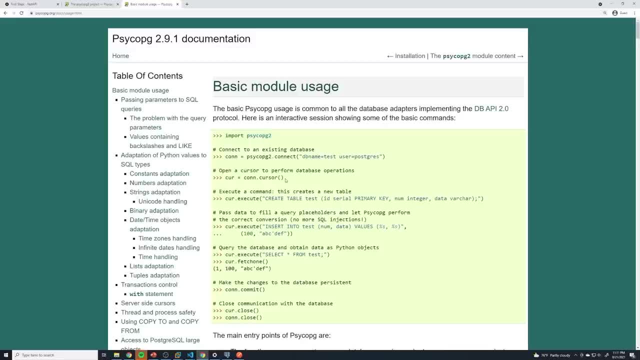 we set up a cursor, So this cursor is what we use to actually execute SQL commands, And so you could just do cursor dot execute. And then here we just say: you know, create table. Well, you guys aren't familiar with that command yet, but you can. 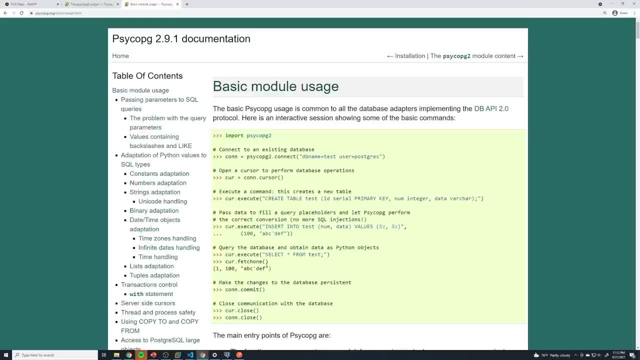 do you know, insert into. you can do select star from test, And then at that point we can then do fetch one, fetch all, And then if you ever want to make changes to a database, you just do commit, So it's. 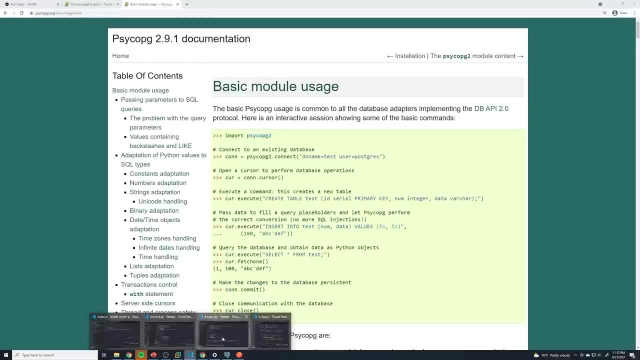 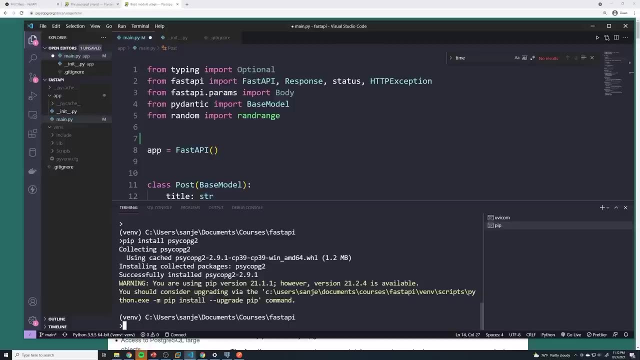 fairly straightforward. So let's go to our code and set this up, And so the first thing that we want to do is we want to install that library. So we'll do pip install And I'll just copy that name. All right, and now it's successfully. 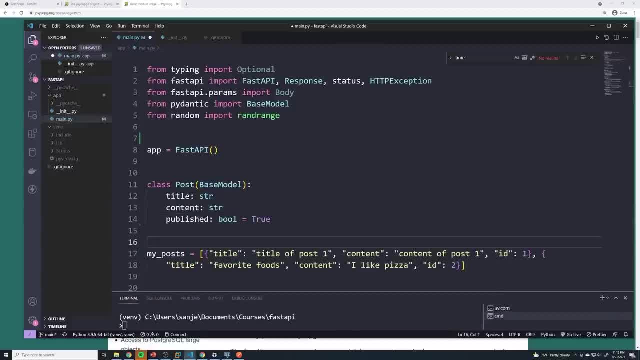 installed, So let's set up our connection, And so a connection to a database can fail right. Maybe the database is unreachable, Maybe the database is down. There's a lot of things that could cause issues with us being able to connect to it. 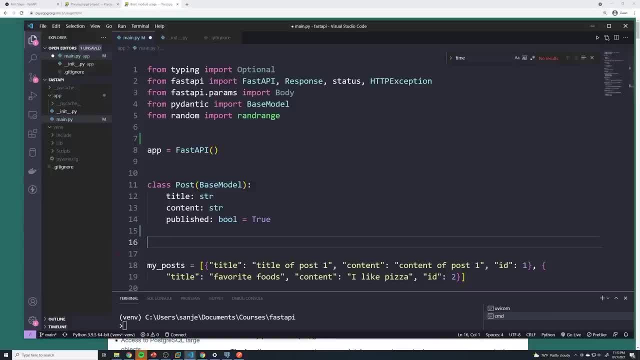 We could put in wrong passwords or something like that. So anytime you have some kind of code within Python that could potentially fail, we're going to use the try statement. So I'm going to say try and then we're going to say connection equals. 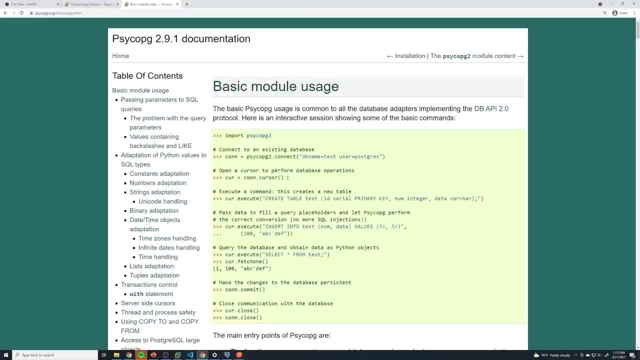 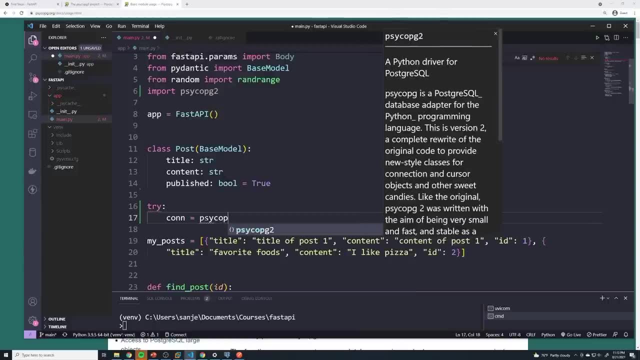 And then I realized the first thing that we have to do is we actually have to import the library. So let's just copy this line right here, And then I'm going to say PSYCOPG2.. I don't know if there's a specific way to actually pronounce that. 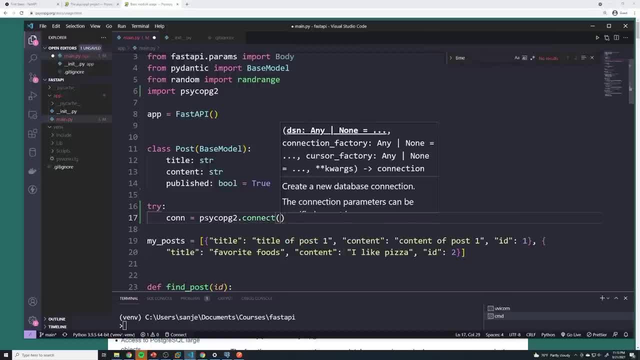 That's why I'm not trying to pronounce it. And then we call it the connect method, And so here we have to pass in a few properties. So the first property is going to be the host. So that's basically the IP address. 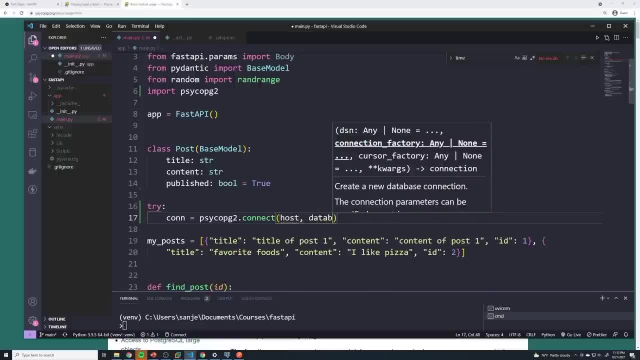 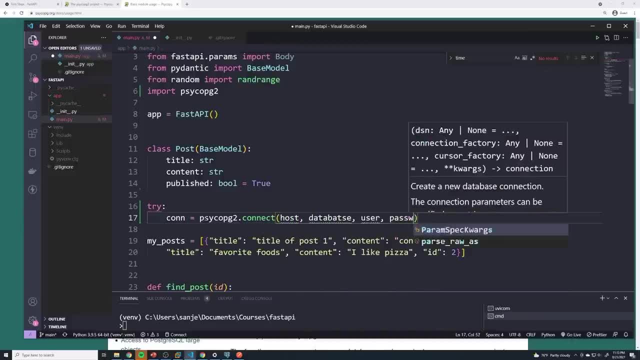 We also have to pass in the specific database we want to connect to. We also need to pass in the username that we want to connect as as well as the password, And for now we'll just keep that as such. So let's. 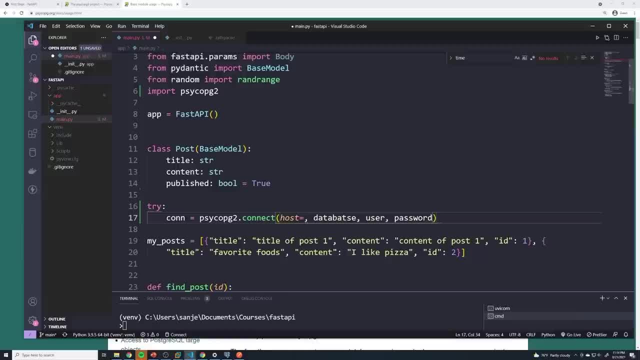 fill in these fields. So what's the host? So, since this host is just our local machine for the IP address, you could just say local host. That means our own IP address. I misspelled database And I'm going to set this to be. 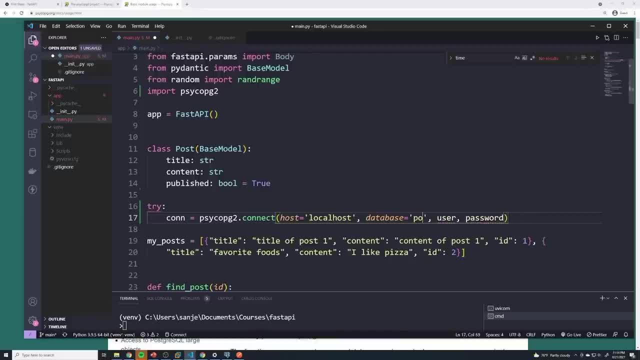 Postgres. because that's what? sorry, it's not going to be Postgres, It's going to be FastAPI, Right, so that database is just going to match up with the name of our database, right here. Username: we've been using the. 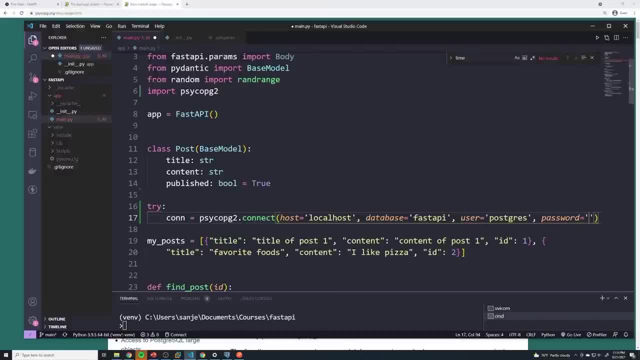 default Postgres username And then password. I'm guessing you guys could have guessed what my password is: It is password123.. Alright, and then, finally, there's one extra thing that we have to pass in, And so this library is a little bit. 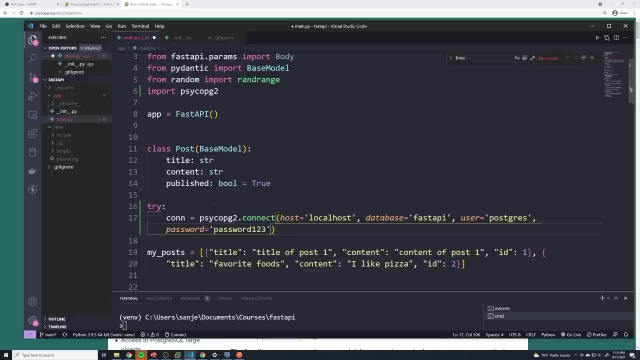 weird. So when you actually make a query to retrieve a bunch of rows from the database, it doesn't include the column names. It just gives you the values of the columns which you know. it's like I don't know what value maps to what columns. So 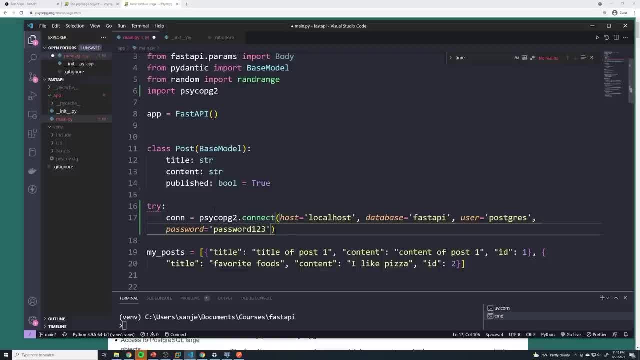 you actually have to pass in an extra field to get the column names, which kind of seems dumb, but that's the way the library works, And so what we're going to do up here is we're going to import. something else We're going to do: import. 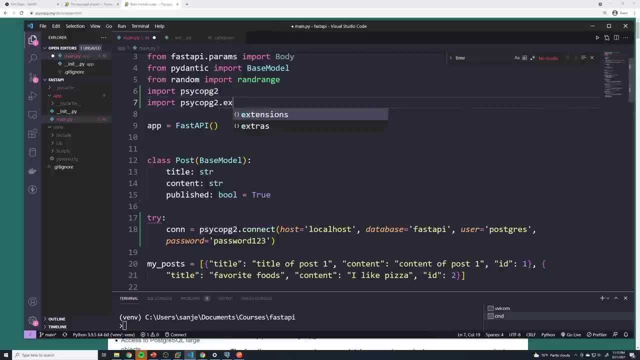 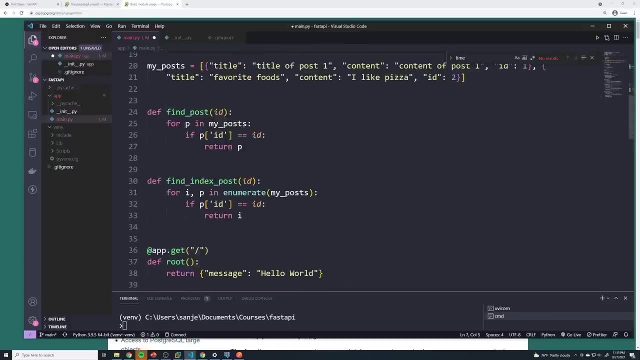 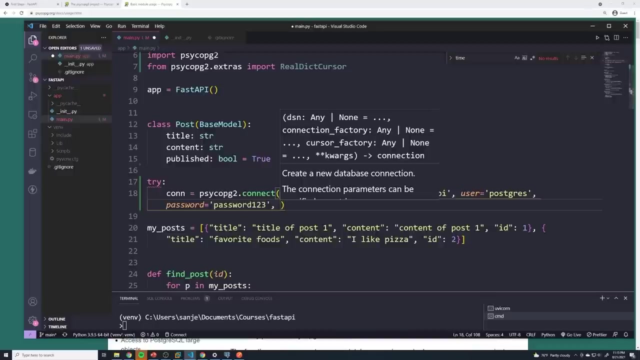 Same library, Dot extras Import, and then real dict cursor, And this should be from. And then the last property we're going to pass in here, the last argument is going to be: cursor factory equals real dict Cursor. So, like I said, all this, 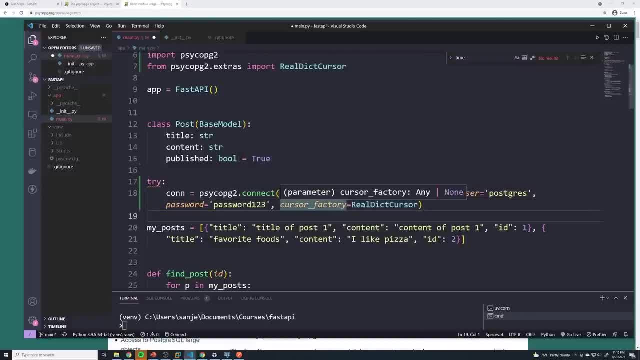 does, is it's also going to give you the column name. It's going to give you the column name as well as the value, So you know which value map to what column. or then it's just trying to figure the order and then mapping it. 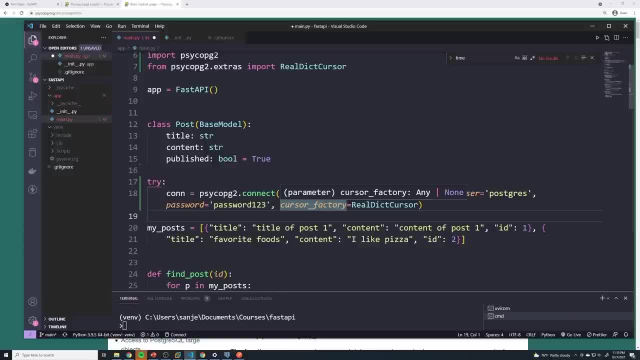 to columns gets a little complicated. So this will just make it a nice Python dictionary. when it returns it, All right, And just like it had in the documentation, we'll say cursor equals con dot cursor. So it's just calling the cursor method and then saving. 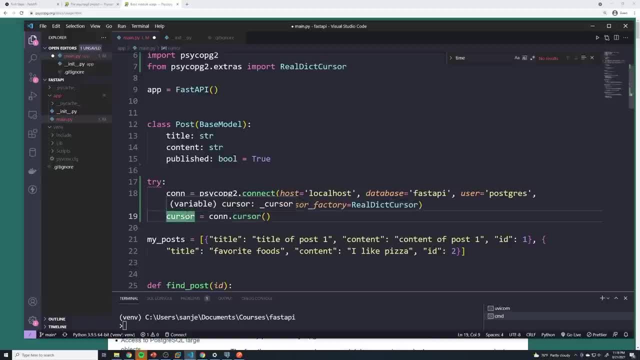 it in a variable named cursor, And so all this is going to do is this is what we're going to use to actually execute SQL statements, And if it's successfully able to connect, we're going to say print, and then we're just going to print out something. 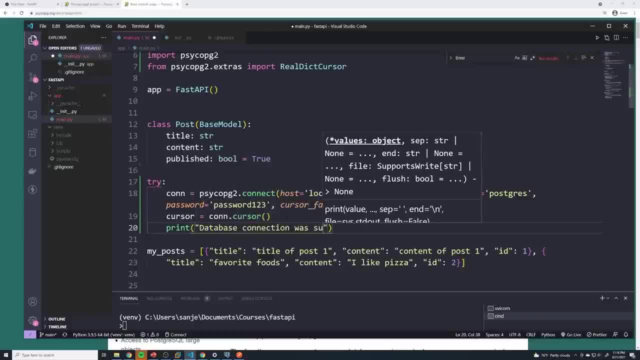 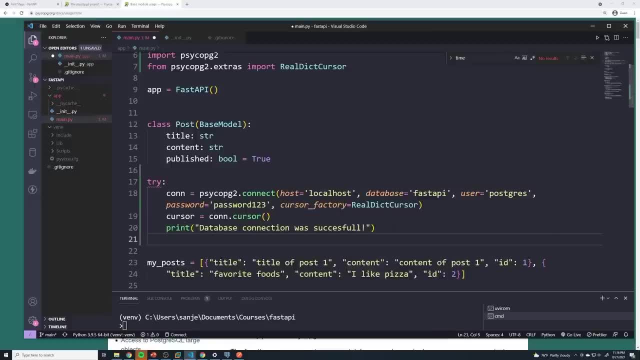 like a database connection was successful. However, if we weren't able to connect to it and we get an exception, we'll say: accept exception as error. So we're going to get the error stored in a variable called error, and then we can just say: 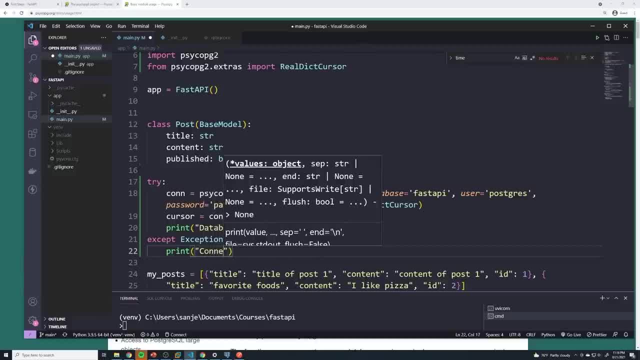 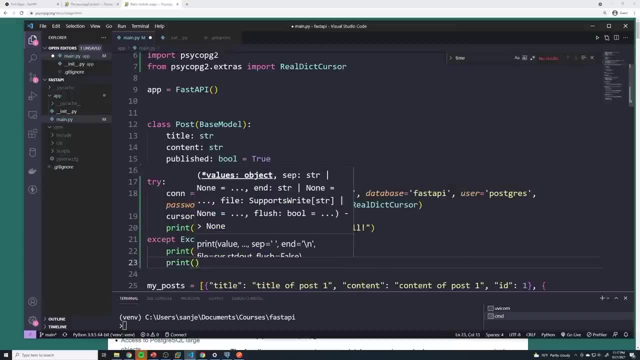 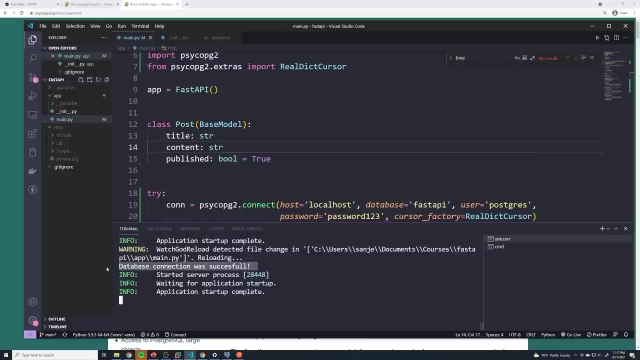 print: connecting to database failed And then after that, just for our knowledge, we can say the error was error. We'll just print out the error. Let's save this, OK, and you can see that we were successfully able to connect to our database. 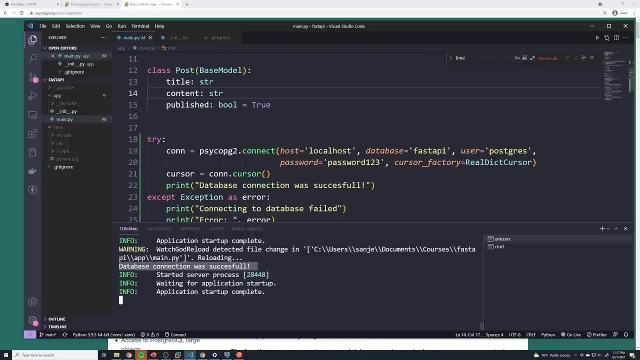 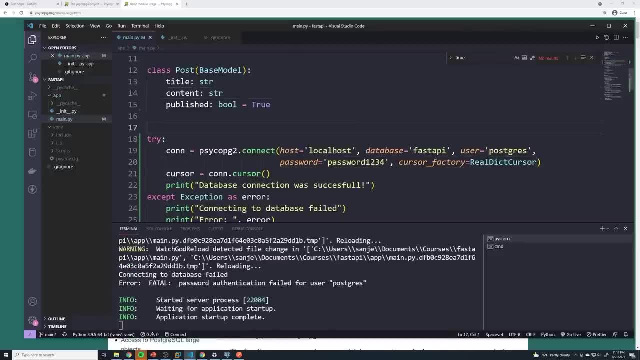 So it looks like everything worked well. But just as a quick test, I'm going to change my password here. I'm going to put it as an incorrect value, So let's save this and let's see what happens. All right, We can see that. 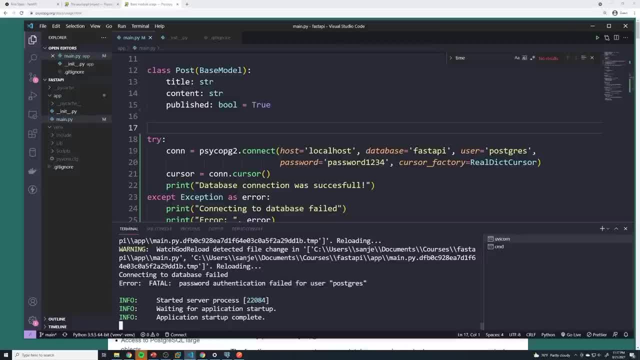 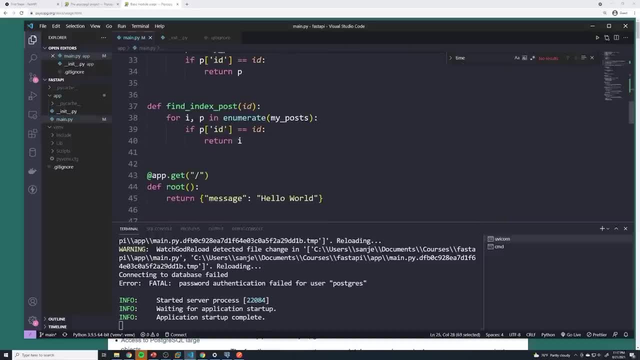 The password failed. And so, at this point, what the code does is it failed, It printed out the error and then it just keeps going through the rest of our code. So then it starts up our fast API server, But at this point, you know, our application is not going to work. 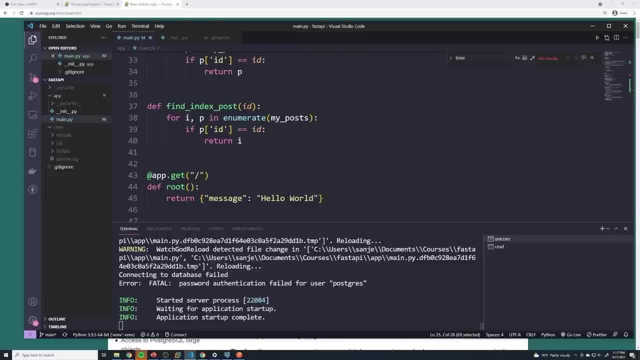 because the Postgres database connection failed. So really our application, our API, our web server can't do anything until we get a connection to our database. So just having it fail and then kind of gracefully handling that error doesn't do anything. We need to wait for that connection. 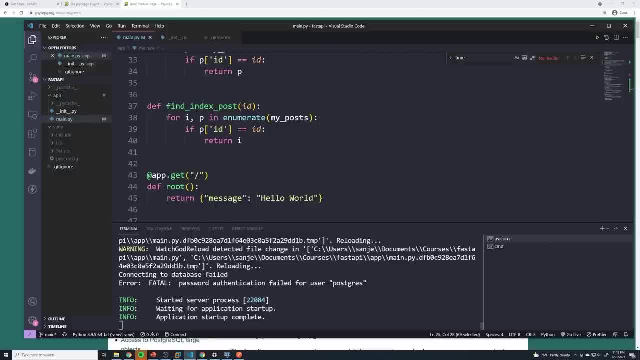 To actually go through before we do anything else, Or then at that point there's really no point in having our server up and running if we can't access our database. So what I like to do is we're going to set up a while loop. 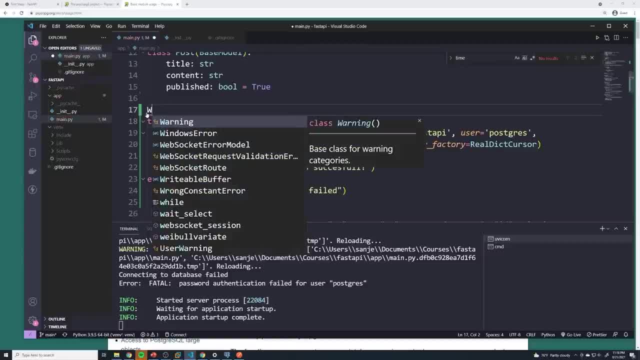 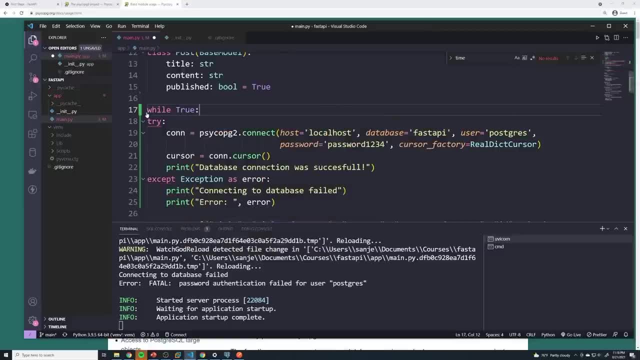 And I'm just going to say while. And I want this loop to just continuously run until we successfully get a connection. So we'll say while true, Which means we're just going to keep doing this over and over and over again until we break out of it. 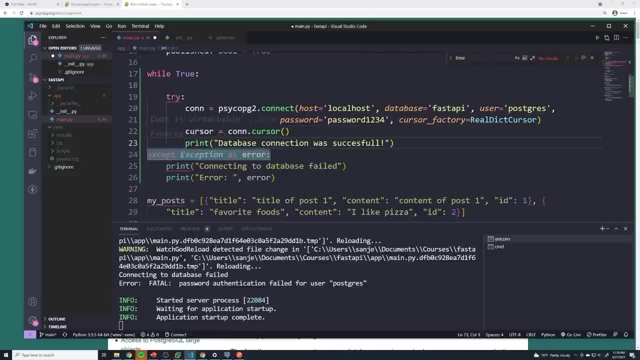 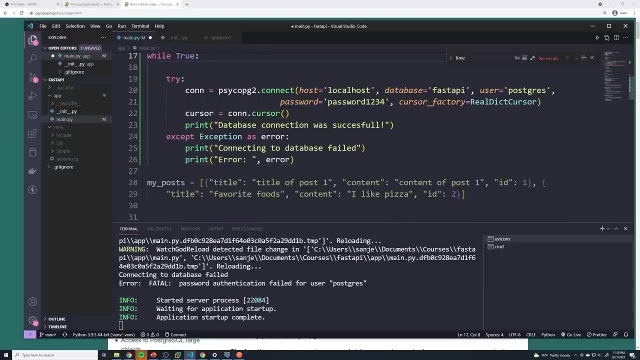 And I'm going to tab everything over. I put everything in that while loop, Alright, and so, while this true if we successfully are able to connect to the database, I'm just going to break out of the while loop. However, if we fail, then it's. 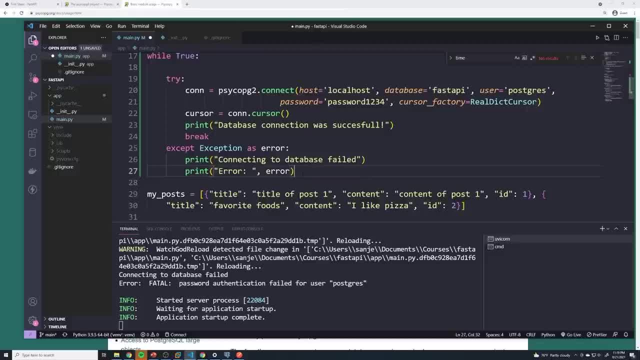 just going to go right back into that loop. And so now one other thing is: it's going to do this really quickly, And I would like for after an error, I would like it to kind of wait two to three seconds before it tries to reconnect. 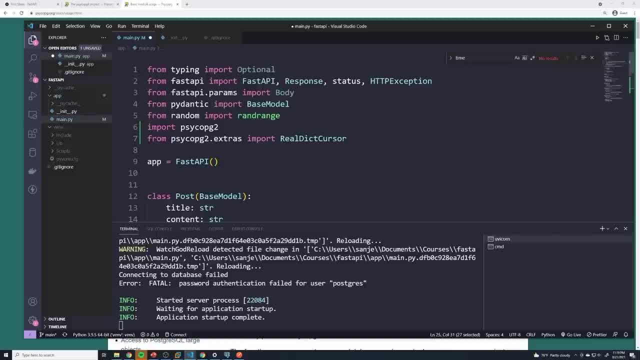 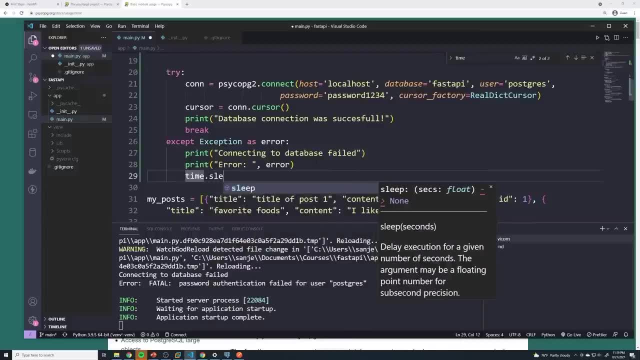 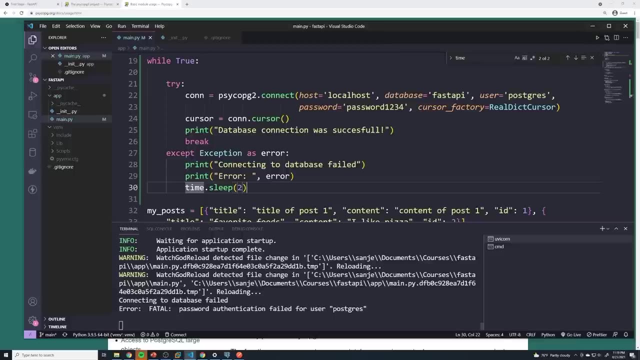 So what we can do is we can import the time module. I'll say import time And here I'll just say timesleep And I'll sleep for two seconds. Use whatever time you want. And so now, if I hit save, check out what. 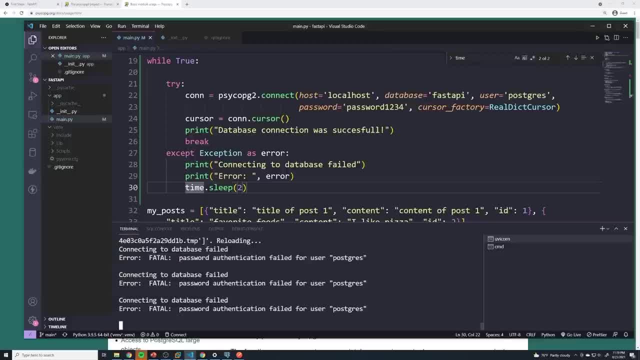 happens. So it failed to connect because of wrong password and then it's just going to keep retrying every two seconds Now for a failed password. it's never going to connect. However, if it's an issue with your internet, if it's an issue with the database having, 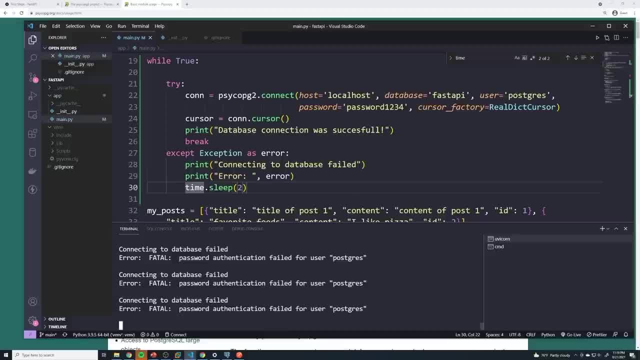 not fully initialized, then having it just kind of redo this until the database fully comes up is a nice way of kind of handling that. So if I change this now back to the correct password, we see that we're now successfully able to connect. 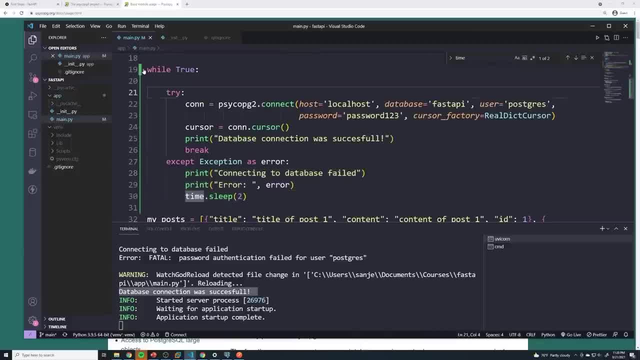 So this is our code for actually connecting to our database, And at this point we can start working on actually writing our SQL code and then you know, being able to manipulate our database from our fast API. And I do want to point out one thing Generally: 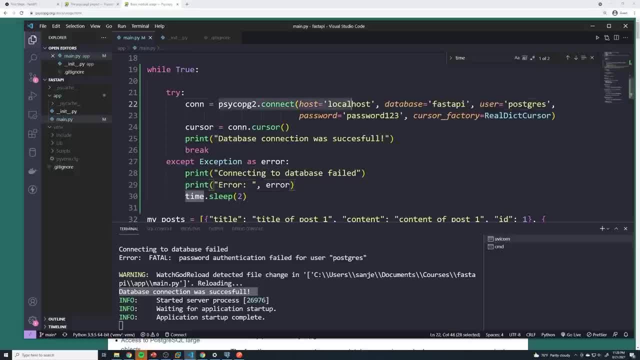 when you're working with your code. what we did right here is very bad. We hard-coded all of our database information right into our code. This creates a problem because, first of all, when we check this into Git now, our database password is stored in there. 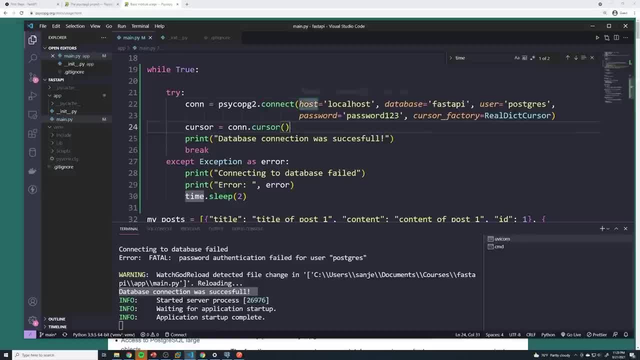 And then we run into some extra issues, because this is the connection for our development environment or our development Postgres server, Our production Postgres server, is not going to be running on a local host. maybe The database might be called something else. The username and the password. 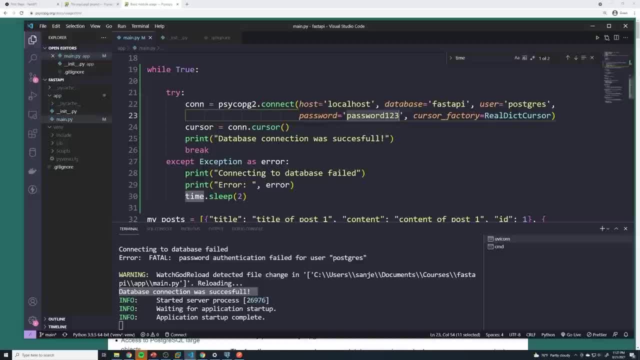 are for sure going to be different. So if we hard-code it in, we won't actually be able to change it in the future. We need a dynamic way to kind of have our code change based off of if it's in our development environment. 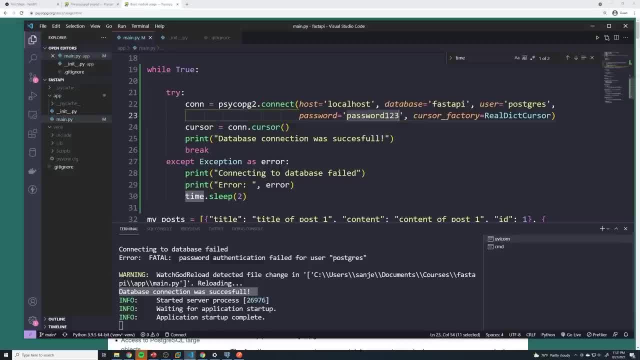 or our production environment. So later on in this course we'll figure out how to do that. However, for now we're just going to work on keeping things simple and just learning how to interact with the database before we start moving into things like 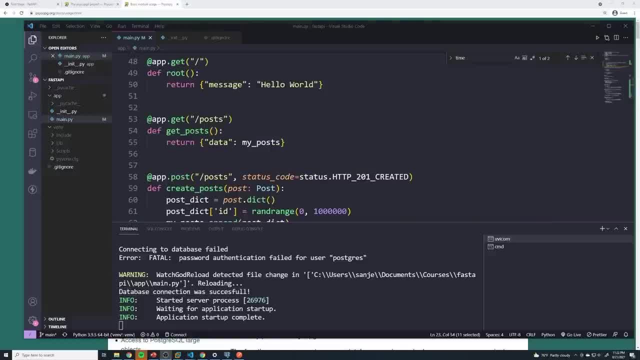 environment variables. Alright, so the first thing that we're going to work on is retrieving all of our posts from our posts table, And so what we're going to do is we'll go to our specific path operation for that, which is the appget slash post. 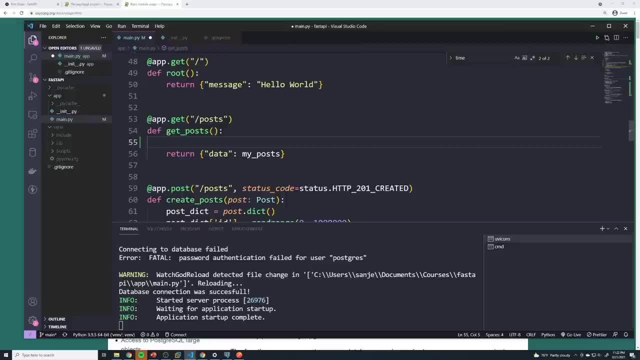 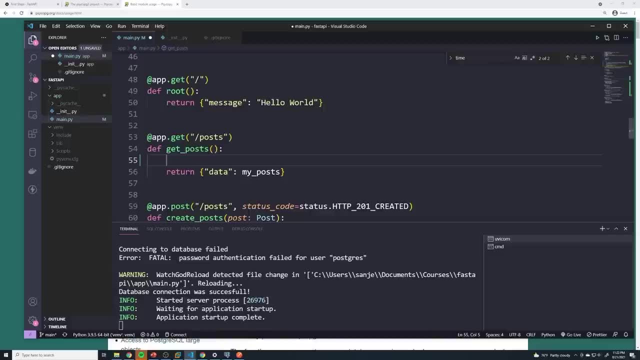 right here And let's figure out how to do this. So if we go back up to our connection right, you'll see that we have access to this object right here, which is cursor. So we're going to use that to actually make a query. We'll. 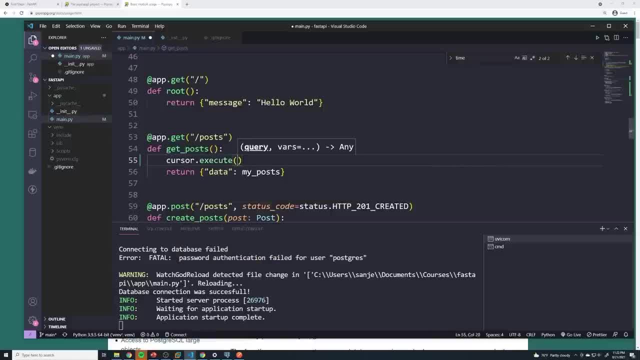 say cursorexecute, And then this is where we are going to paste in our SQL statements. So I'm just going to put in three quotes right here and then we just put in our SQL statement. So, in this case, right to retrieve all posts, we just do select. 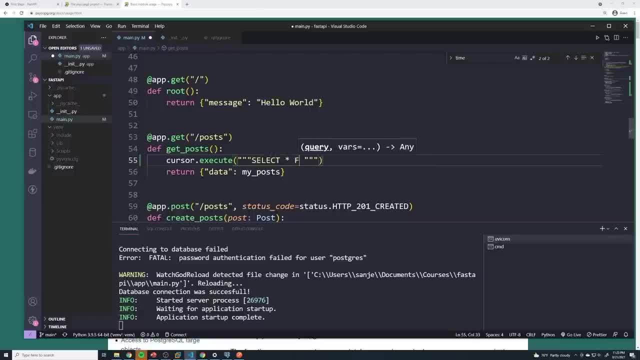 star from posts. Okay, and let's save this as a variable. So I'll just say these are my posts, And then let's just do a print post to see what we get. And so I'm just going to go to my postman and we'll just 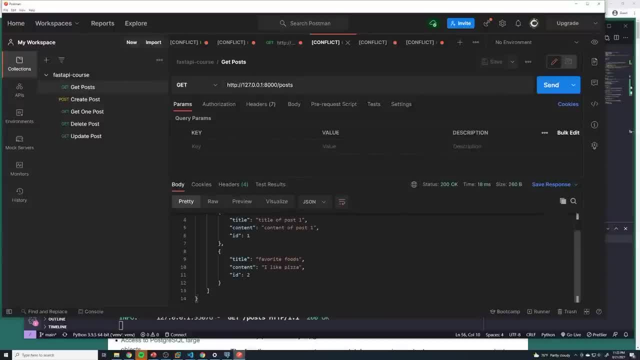 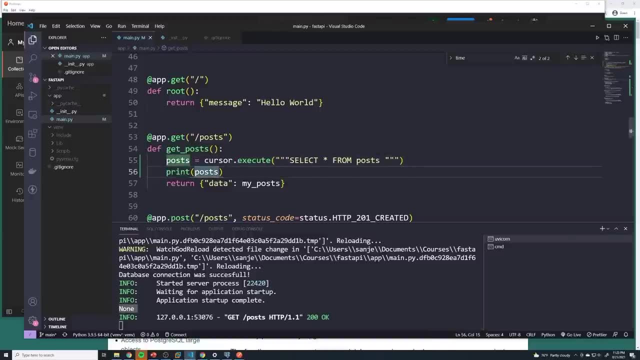 find my get posts request. We'll send it All right and let's see what happens. right, We can see that it printed out none, So this doesn't actually do anything right? This is just passing in our SQL statement, However, to actually run it. 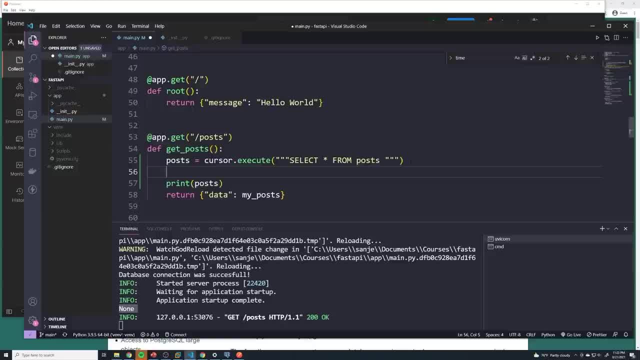 we have to do cursor dot and then we have a couple of options. We can do fetch all, fetch many, fetch one. So when it comes to retrieving multiple posts, we're going to always use fetch all. Don't worry about fetch many. I don't think we're. 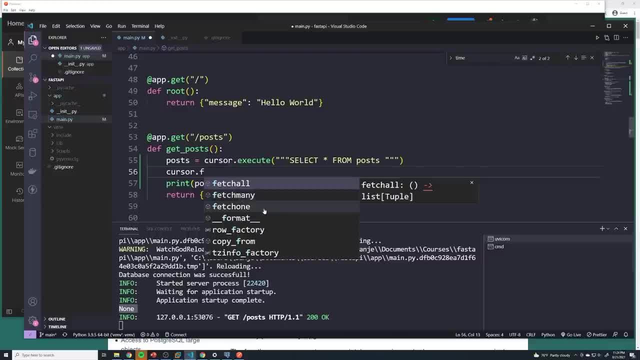 ever going to use that. And then if we ever want to find one individual post- you know like finding a post by an ID or something- then we can use fetch one, Because I believe if you want to fetch a post by an ID and you do fetch all it'll technically get. 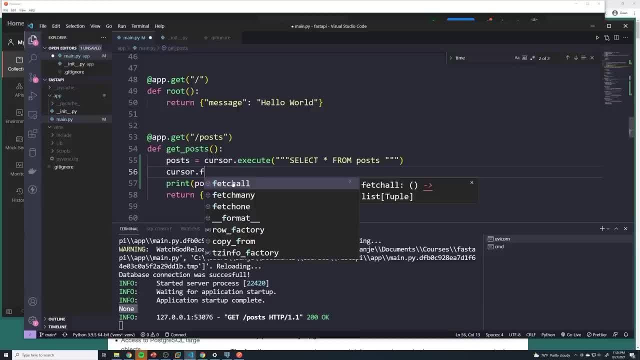 it, but it'll just keep searching through the database for another post with that ID. However, we know that only one post can have that exact ID. so it's inefficient to kind of search through the entire database when we know there's only ever going to be one result. So for those 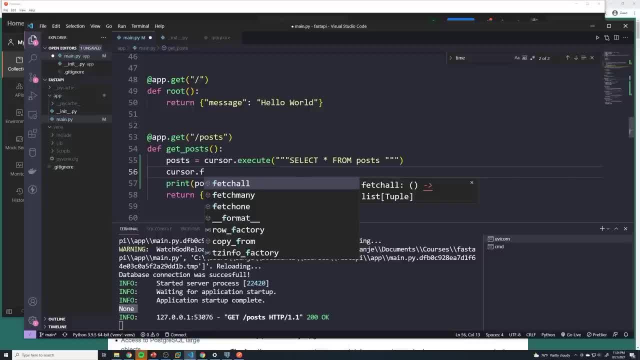 it's always better to use fetch one, but since we're retrieving multiple posts, we're going to use fetch all. And at this point you know we don't actually need to save this in a variable, because it's never going to return anything. We can save the output. 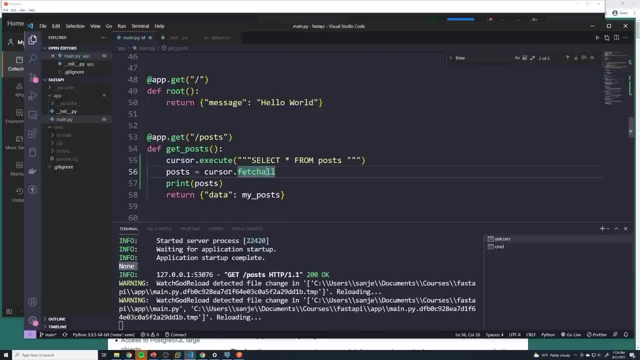 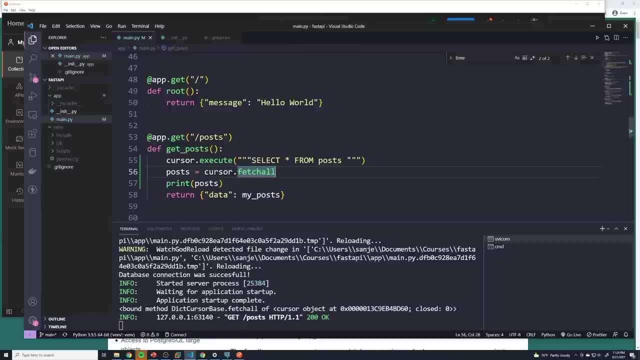 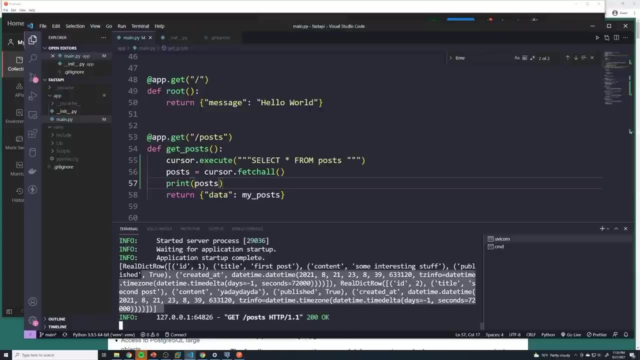 of this to be posts. So now, if we save this, run this again and I realized I forgot to actually call it. Let's try that again. Right, you can see that we got all of our posts from here, And so now. 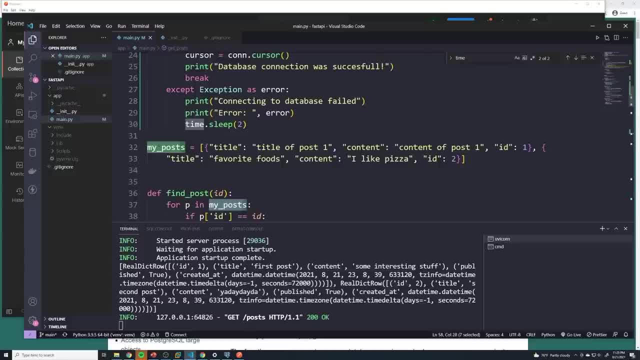 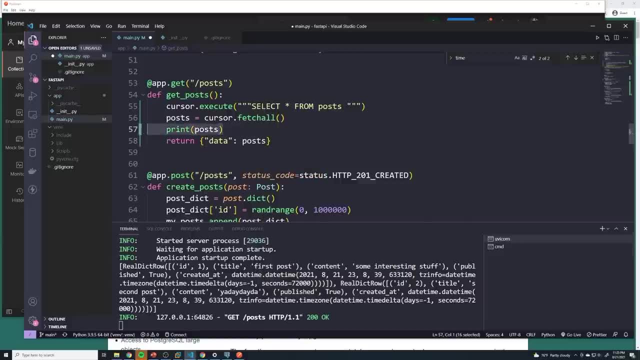 instead of returning my post, which is our old array which we're not going to use, we're going to return what we just fetched. So we're going to return posts And we'll go rid of that print statement. It's not. 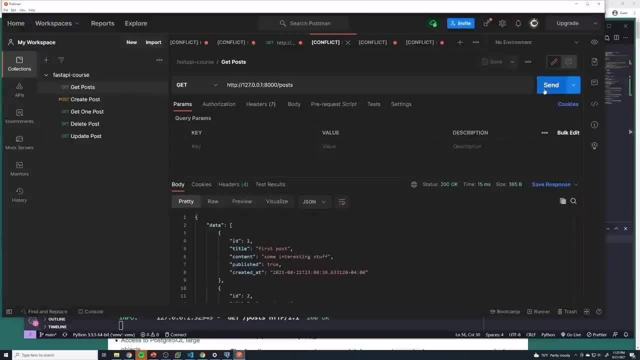 needed anymore, And hopefully this works. So let's hit send. All right. and so now you can see we've got our two posts from our database And it's got all the extra fields. So it's got the publish, which is the default value, and then it's got the 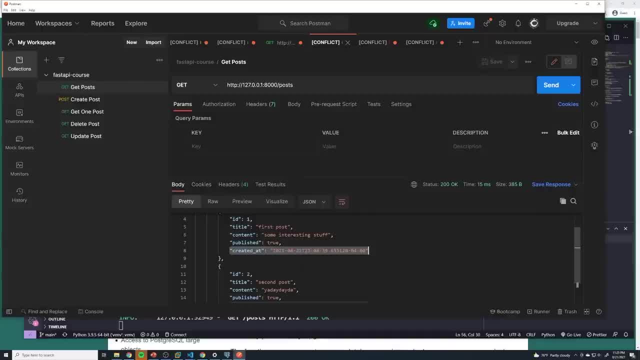 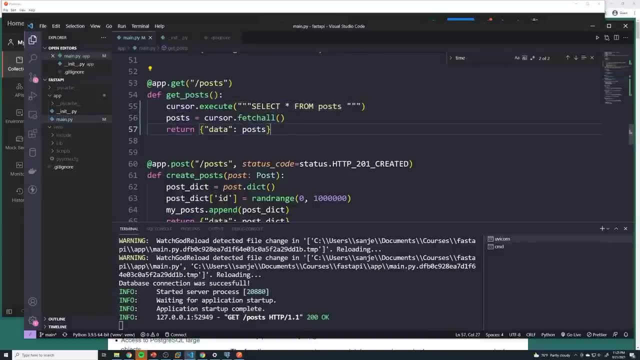 created at timestamp, which Postgres added. So now we've actually successfully been able to retrieve posts from our Postgres database And you can see how easy it is to actually work with that. In fact, it was actually a little bit easier to do this. 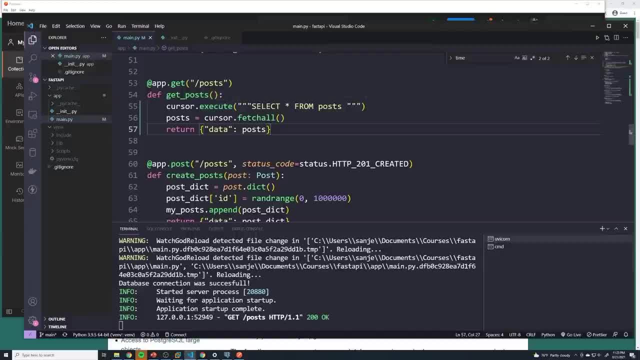 than to actually work with just an array stored in memory. It really just comes down to understanding SQL, And since we spent the last half an hour or so really drilling into how SQL works, you'll see that SQL is pretty easy. And then, once you know SQL, 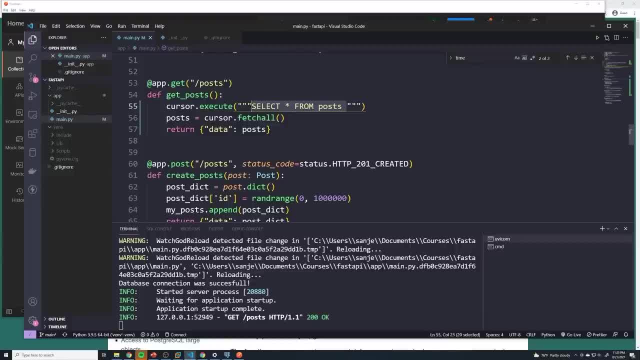 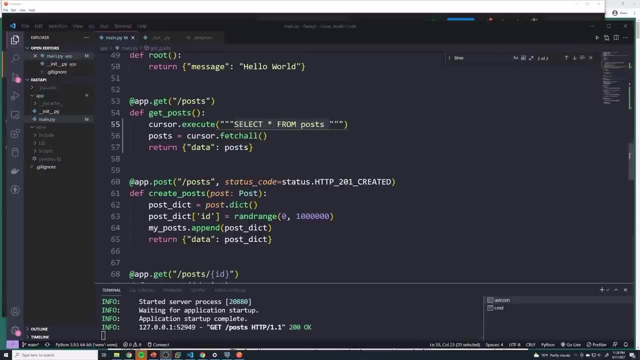 fetching, retrieving, updating, deleting posts from a SQL database- it's even within your Python code- is dead simple. Okay, so let's now move on to creating a brand new post, And so, if we just quickly take a look at the code, that we have right. 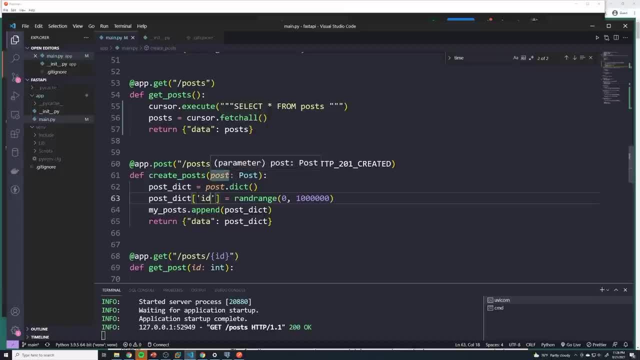 here you can see that we have our schema. we're going to save that in our Pydantic model, and so we'll be able to access the properties from the body within this post object. So I'm going to clear this out and just delete all of that code for now. 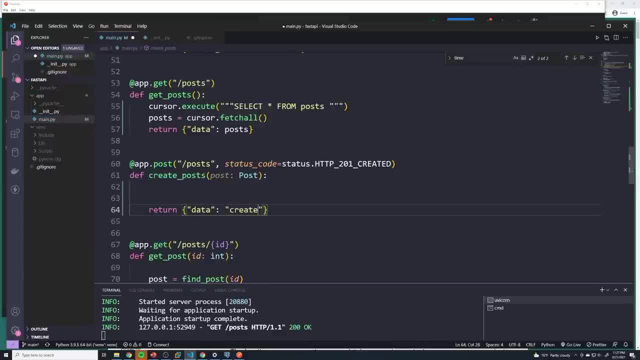 And for now I'm just going to hard code some value. I'll just say: created post, And so let's work on inserting a new post into our database. So once again, we're going to access the cursor object. We're going to do: 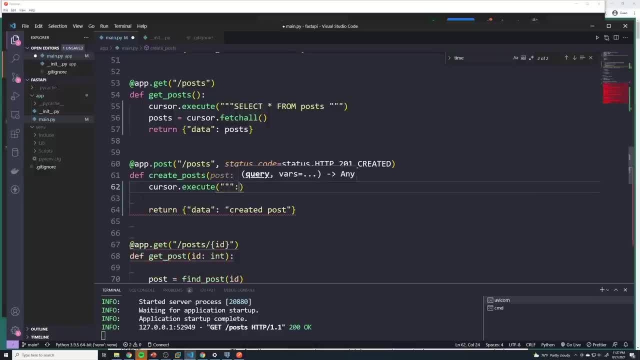 cursorexecute And then, once again, we're going to use the three quotes And we're going to use typical SQL. So to insert something into our database, we do insert And then we say: insert into What table do we want to insert it into? I'll say the. 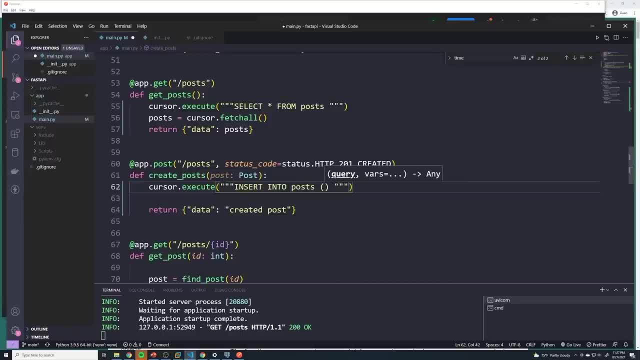 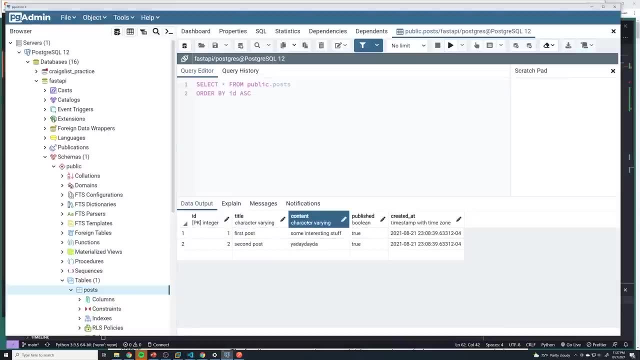 post table And then here we have to pass in the columns of all the fields that we want to enter in. So if we go look at our database, we have to pass in a title and a content And then everything else is optional. So we can. 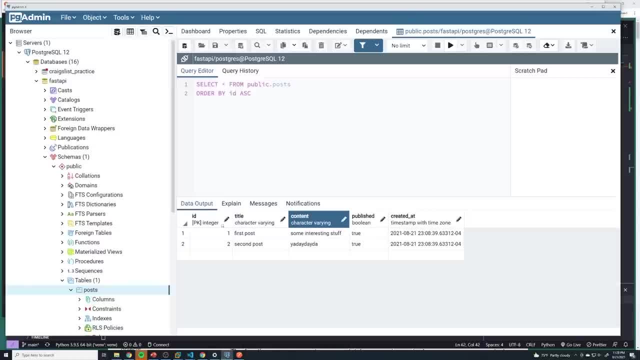 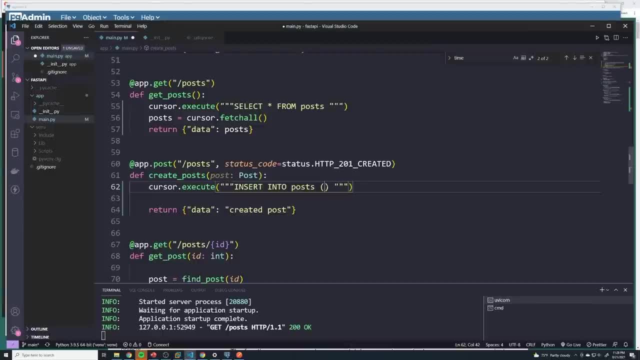 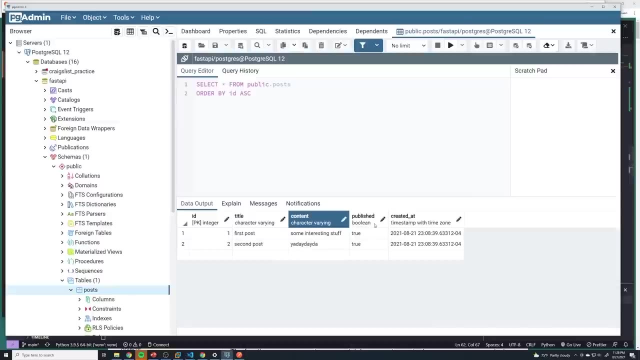 also provide published as well, And then the database creates the created at and the ID. So it's really just these three columns that we're going to pass into here, And so it's going to be title content and then published Yep, And then we have to. 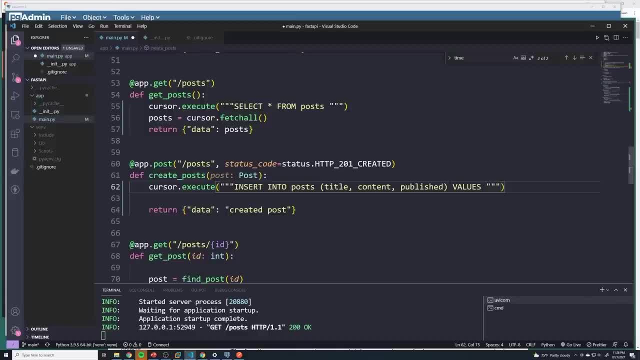 pass in the values for those columns. And this is where things get interesting. You never want to do any kind of string interpolation and then pass in the values of posted directly into this Instead. what we want to do is we're going to parameterize. 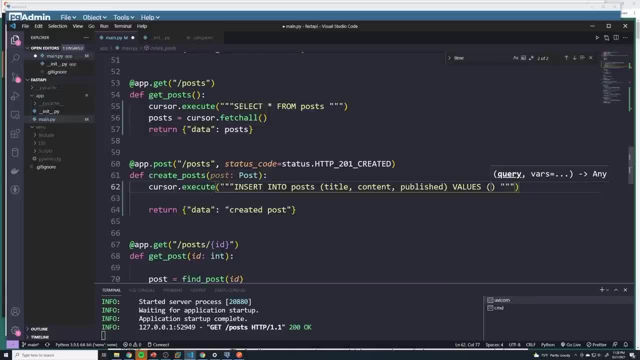 or sanitize all the data that we put into this Equal statement. So what you should do is do percent S, And so this kind of represents a variable, And we're going to do percent S and then percent S, And so this variable is. 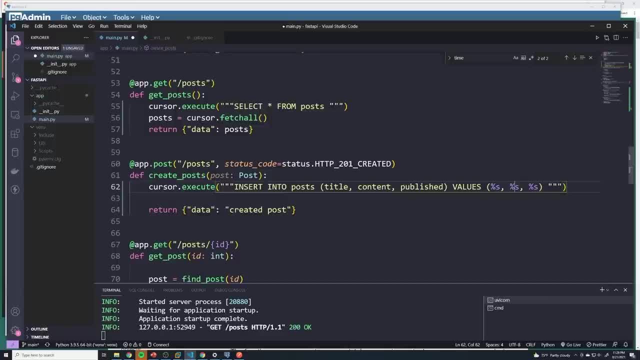 going to be the value that gets passed in title. This variable is going to be the one that gets passed into content And this variable is the one that gets passed into the published column And what we want to set these as we're going to actually use a second. 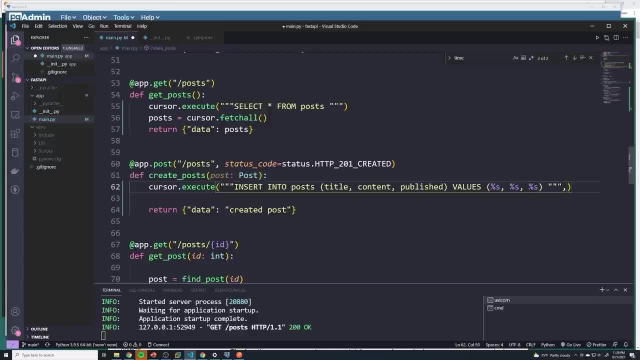 item that we pass into the execute command, the execute method, And so here we pass in the actual values. So this first percent S, what do we want that to be? That's going to be posttitle, So we're grabbing the title. 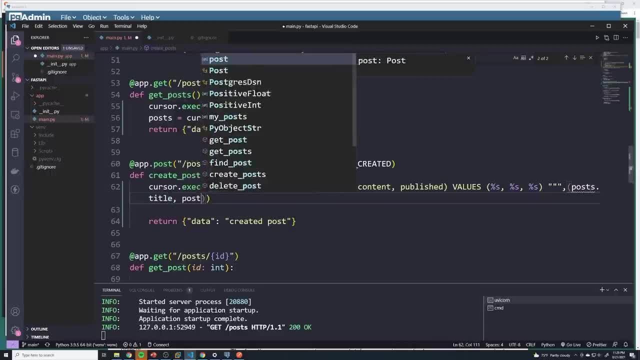 from the body. Then we want to pass in postcontent, And then we want to pass in postpublished. Alright, And this may seem a little confusing, And let me correct that Because I'm sure a lot of you thought we could just do. 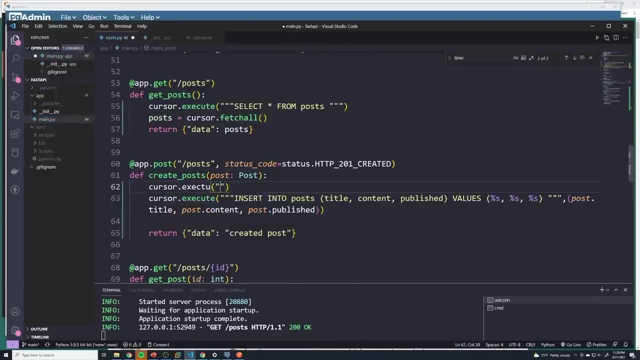 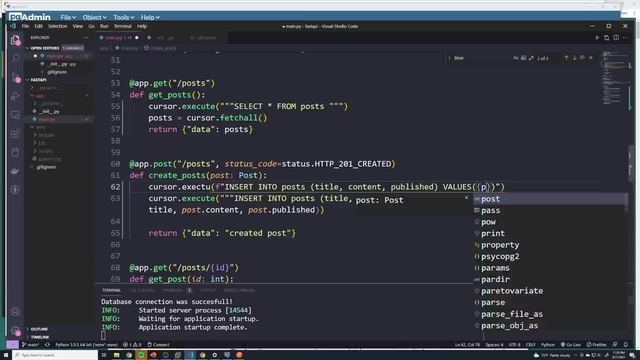 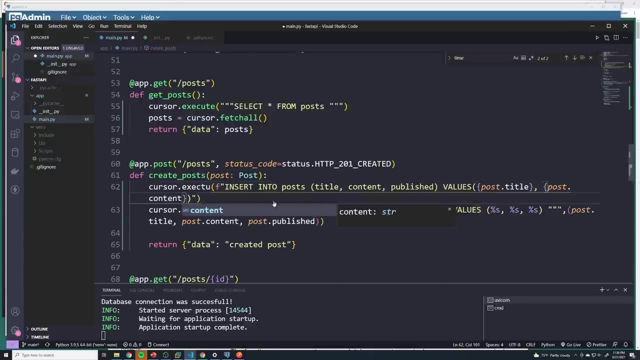 cursorexecute And then here we pass in just an F String And then I can just copy all of this And then pass in here And the values. we can just do posttitle And then postcontent and so on, And this would technically work. However, 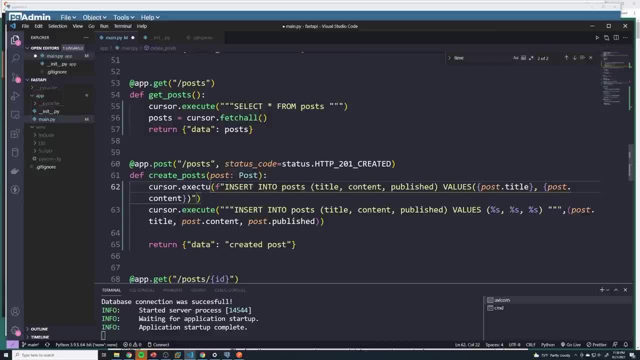 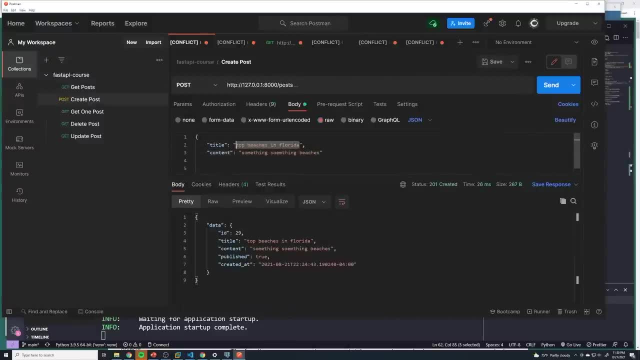 this makes you vulnerable to SQL injection. So if the user for the title decided to, if we go to the create post and for the title he decided to pass in some kind of weird SQL statement like insert into blah blah blah, He puts in SQL instead of a valid. 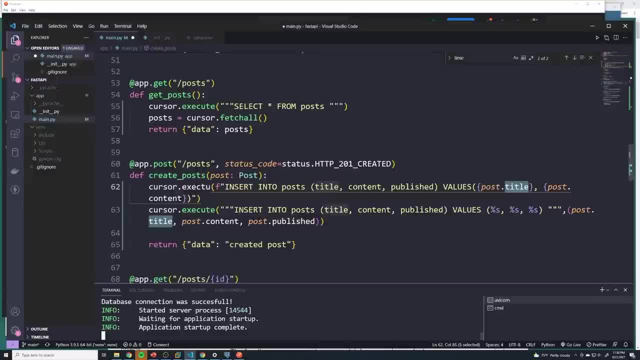 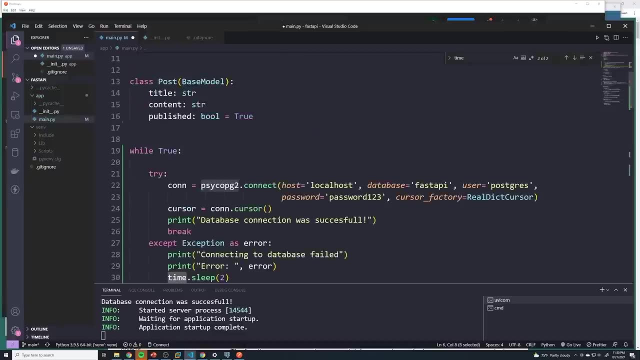 title. This is what is a SQL injection attack, And he could potentially manipulate data within our SQL database. That's why it's never good to pass that data in directly into here. Instead, all of these SQL libraries, like our Postgres library- here They actually 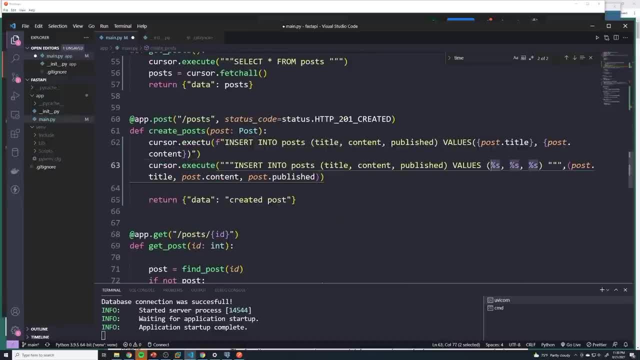 can sanitize the inputs. So when we do this %s method and then pass it in as the second field into the execute statement, It'll actually make sure that there's no you know weird SQL commands in there And it's going to make sure that we're not vulnerable. 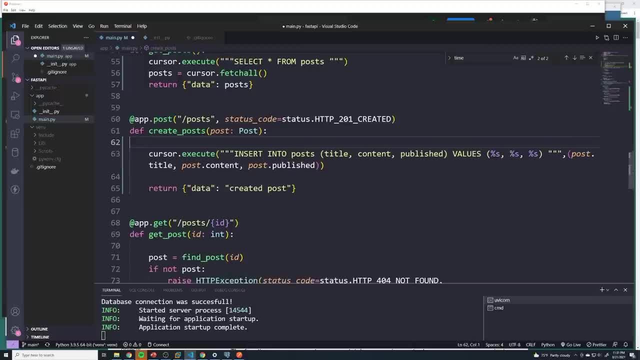 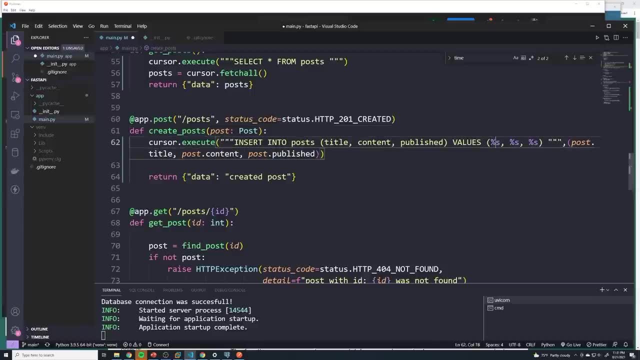 to SQL injection. So that's why we never do it like this And we always do it like this. And just keep in mind: right, these are just variables or placeholders, And then the values we want to pass into that will be passed into these. 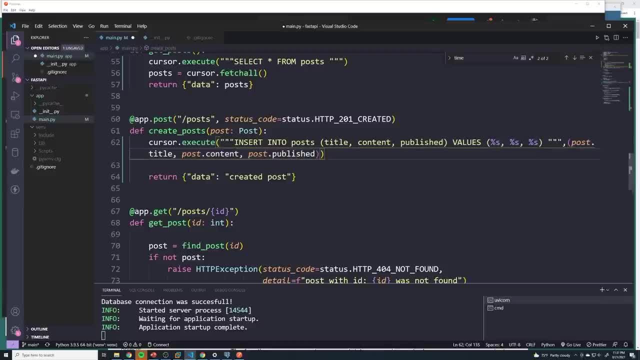 parentheses right here- as the second parameter into the execute method. So postcontent- posttitle- since it's the first one in this list- is going to go to the first %s, and then postcontent is going to go to the second %s and then postpublished will go to the third %s. 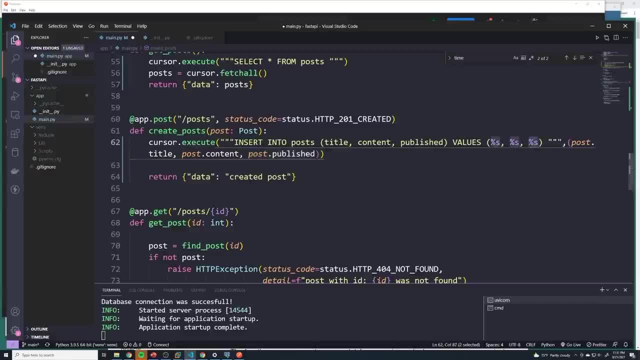 So the order matters. They match up with whichever %s comes first. So if I took, you know, postpublished right and then moved it all the way to the front, well now, postpublished would go to the first %s. posttitle would go to the. 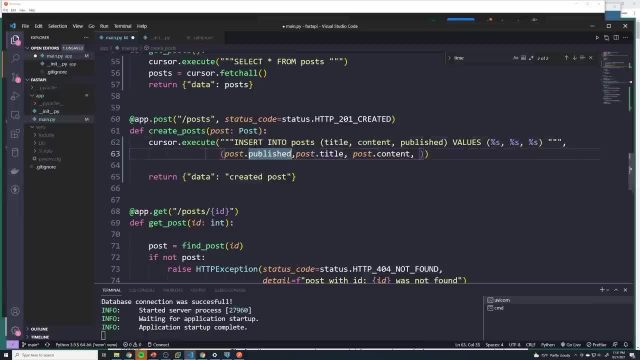 second one. That would cause issues because it doesn't line up with that. So that's why we want to make sure that the order really does, in fact, matter And, just like we had before, anytime we create something in our database, we want to return. 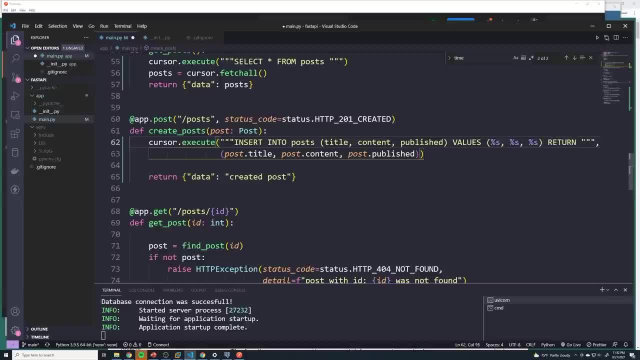 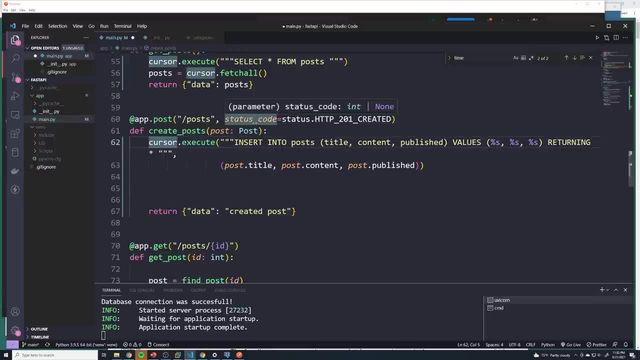 the created result, so we can use the returning keyword And we'll return everything. And so you're probably thinking: you know, we can just save new underscore, post equals that, and then, since we're returning it, it's going to get stored into that variable, and that's not exactly. 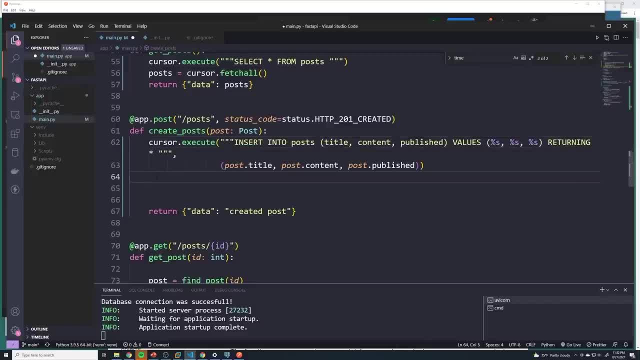 correct. Instead, what we have to do is to get that returned value. we have to do a new underscore post and then we do cursor dot fetch one So that'll get whatever we return from here. And then what we're going to do is we're going to say: 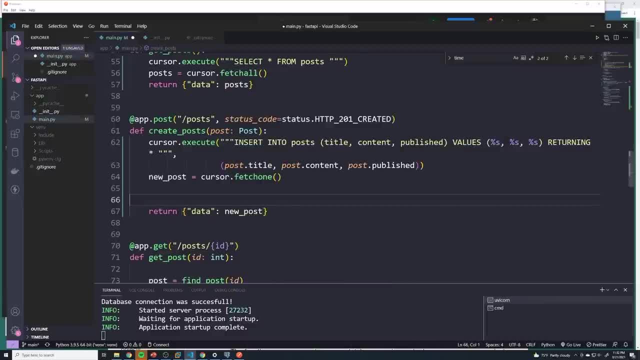 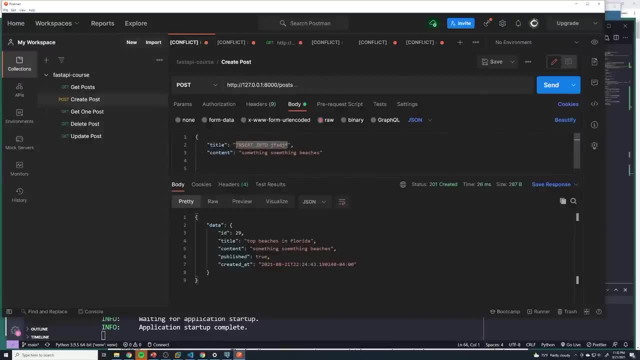 new underscore post is going to get returned to the user. Let's save that and let's see what happens. So go to our create post and then I'm going to clear that out and just say, hey, this is my new post And let's hit send. 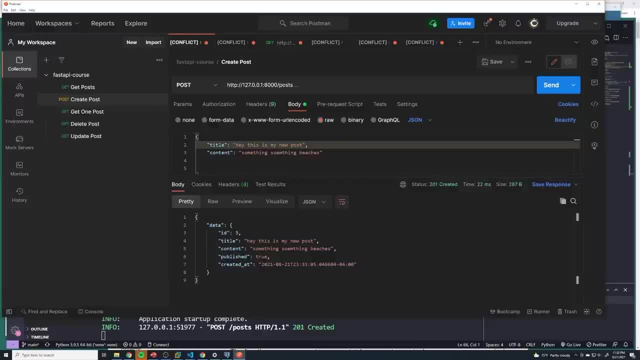 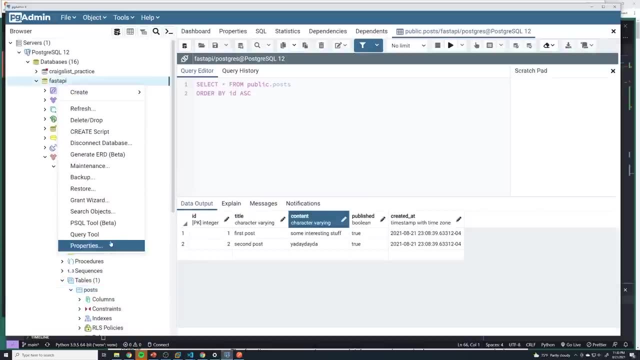 So it looks like everything worked right. 201 created- you can see it's got all of these values. Let's go back to our SQL database. I'm going to just do a quick query, so I'll just say query tool and I'll just say select. 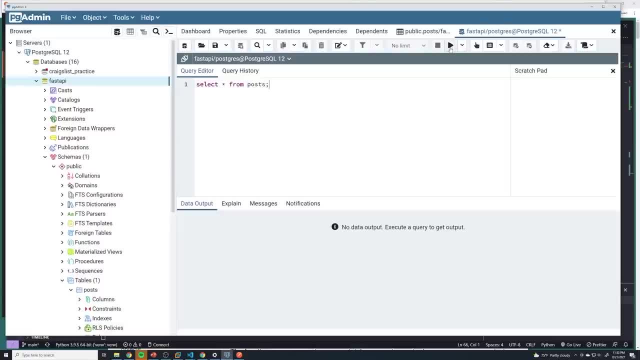 star from posts. Let's run it and if we take a look at the values, and the title should be: hey, this is my new post with an ID of 3. you can see it's not in there And so you might be wondering. well, you know the output. 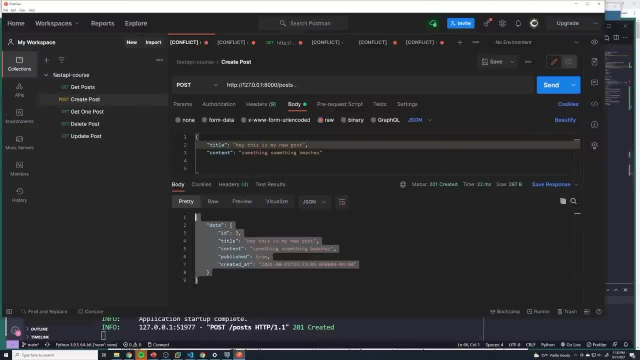 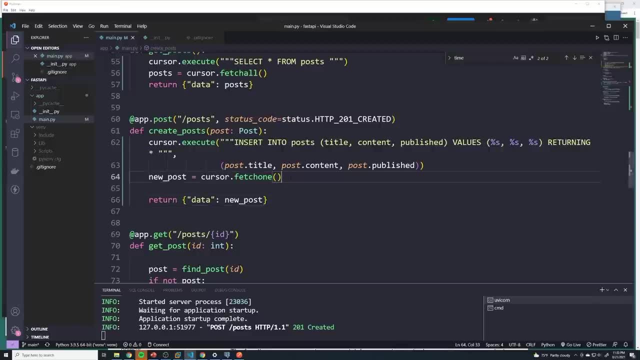 of our API looks perfect. It sent it all back. Well, when you're working with Postgres or any of these libraries, you have to actually do one last thing. You actually have to commit the changes, Just like when it comes to working in our database. you know if I create something. 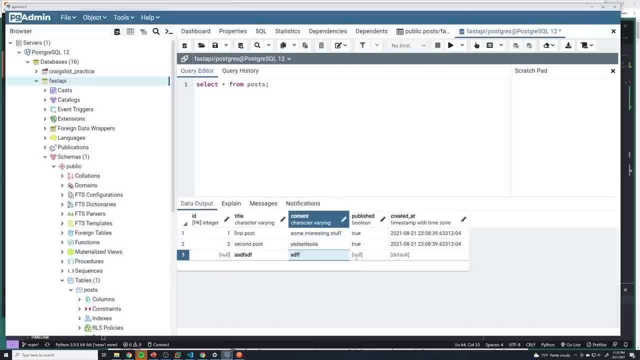 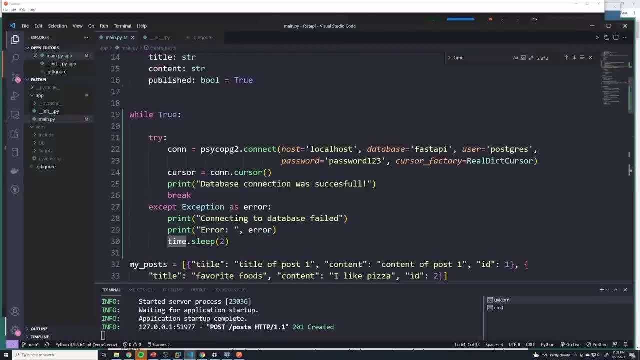 here passing some data into the content. it's not saved in there. I actually have to finally save it. So to save that data we have to reference- instead of the cursor we're going to reference the connection and then we have to do a commit. so if we go down, 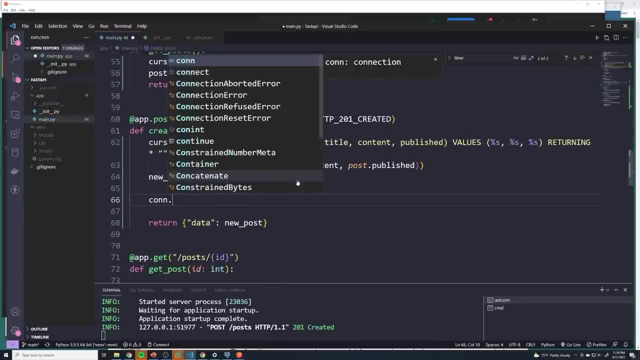 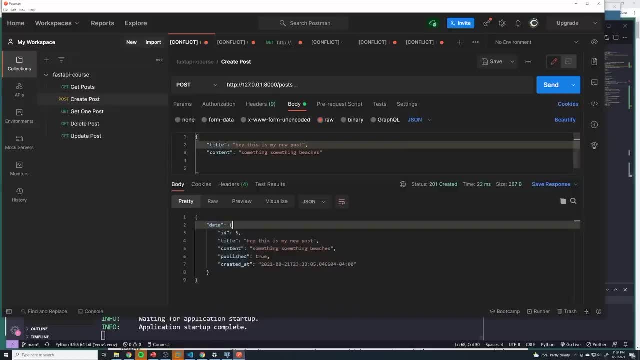 here we just say con, which is my connection to my database, and just say commit. So that's actually going to push those changes out. So we'll save that Now. I'll try this again, Alright, and so now we got it. looks like it has an ID. 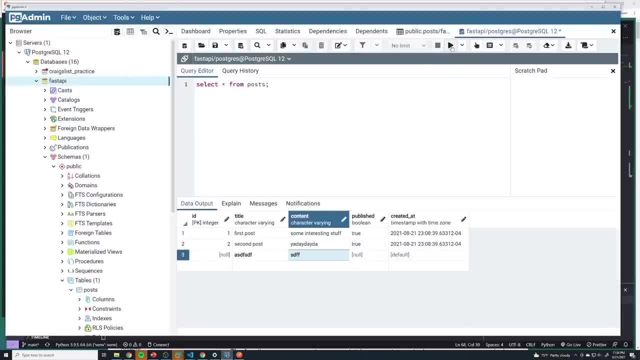 of 4.. If I go to my Postgres database, I'm going to do another search. sure, it's okay if it deletes it, And so now we can see ID of 4. hey, this is my new post, So now it worked, So keep in mind. 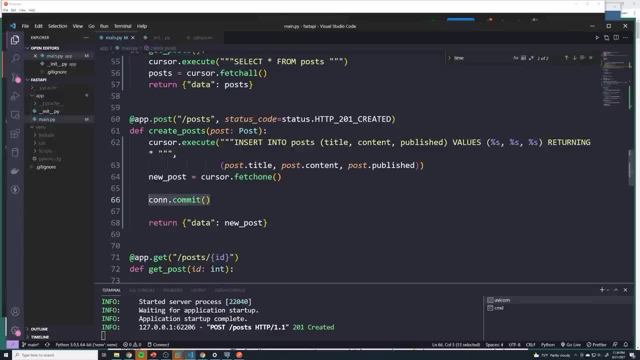 anytime you want to insert data into your code, make sure you do a connectioncommit to actually save it into the Postgres database, because these are all staged changes, So we're staging it. we can see the result of the stage, but we have to commit it to the 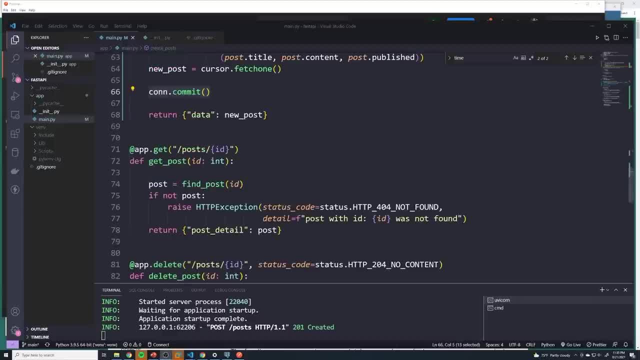 database to actually finalize those changes. Alright, so now let's move on to fetching an individual post by an ID. I want you guys to take a crack at this. see if you can try to figure it out. It's going to be relatively similar to the. 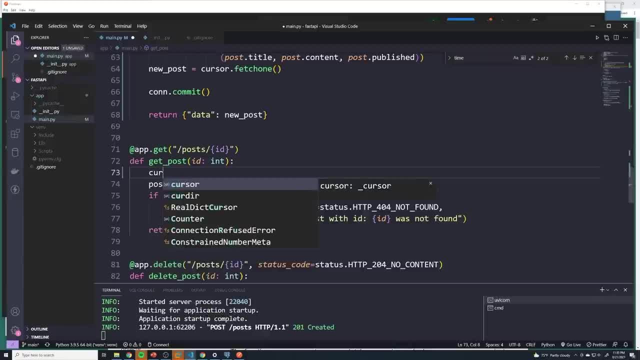 two other previous ones we've done. So we'll start out by referencing the cursor object as usual, and then we'll execute, And then here we're going to pass in our SQL statement And so we're going to do a select star from post. 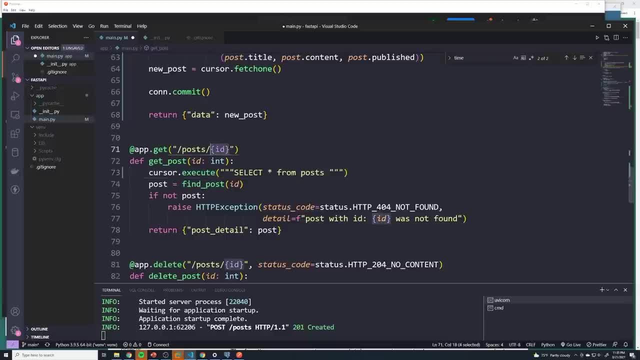 that's going to grab every post, but we want to grab just one post based off of the ID, And so you guys already know how to do that. we can say where ID equals and then whatever ID that you want. And so let's take a look at our database. 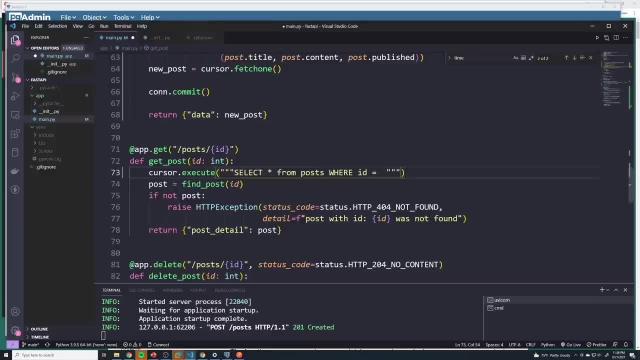 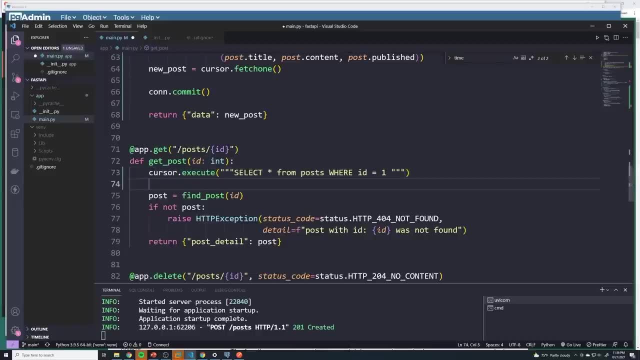 I have a post with an ID of 1. so right now I'm just going to hard code it. I'm going to say: post with an ID of 1 and at this point this is not going to return anything. To actually return something, we'll say: 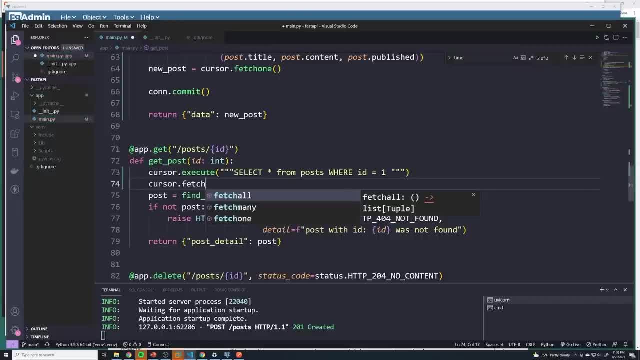 cursor dot fetch, and then we're going to use not fetch all, but fetch 1, because there's only ever going to be a post with an ID of 1, and so this is going to make it a little bit more efficient, and then I'm going to save that. 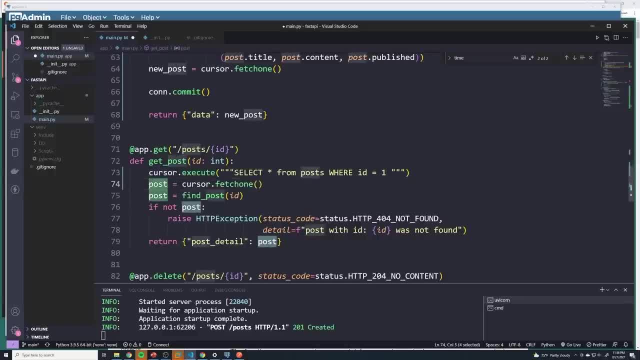 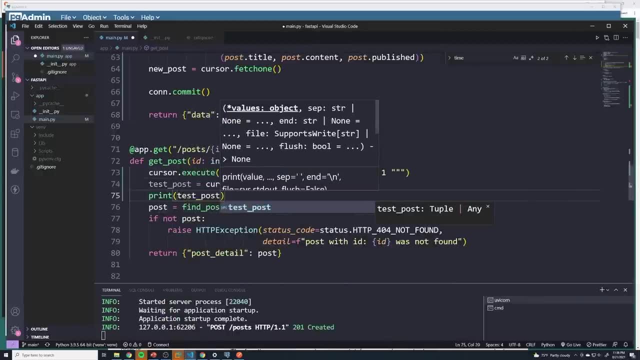 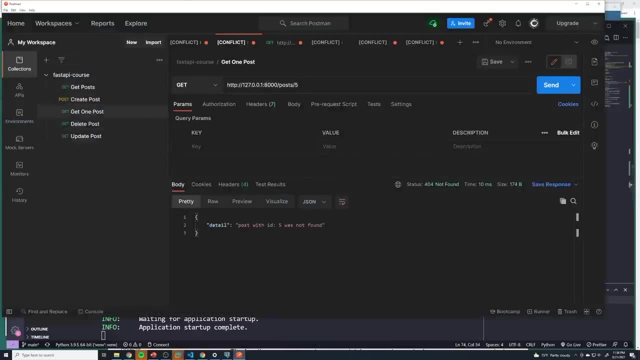 as post- I'll just say test post not to get confused with the other post- And then we're going to print that out just to see if it worked. So let's get one post and it doesn't really matter what we send it as. 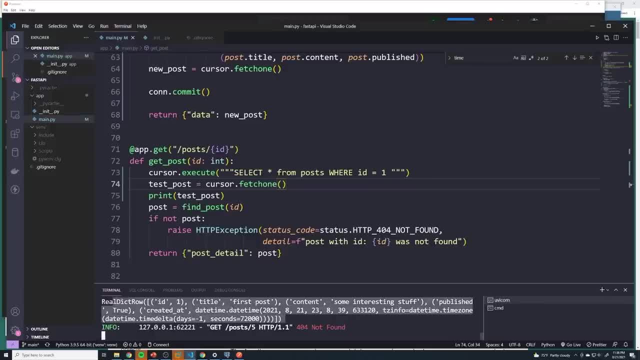 If I take a look at this print statement, you can see that we were able to get just that one single post, So it looks like that worked. so now let's clear out all of this other code. I'm going to remove the print statement actually before we do that. first of all, 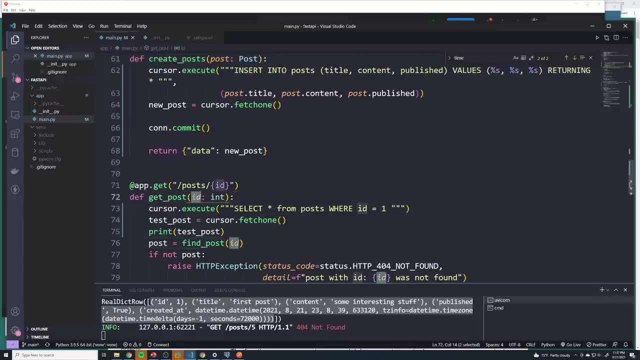 let's not hard code the value anymore. instead, we want to use the ID that we passed in from the path parameter. So how do we do that? We want to always make sure that we're not vulnerable to SQL injection attacks, so we'll do %s. 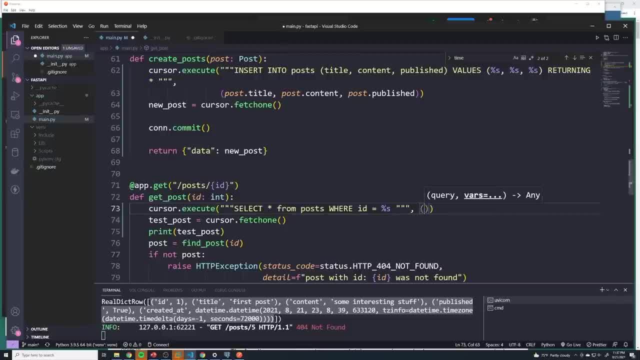 that's going to be the placeholder for the value, and then the second thing that we pass into the execute method: this is going to be the ID. So we take the ID and then that's going to get pushed into this value. So it's essentially doing the same exact thing. 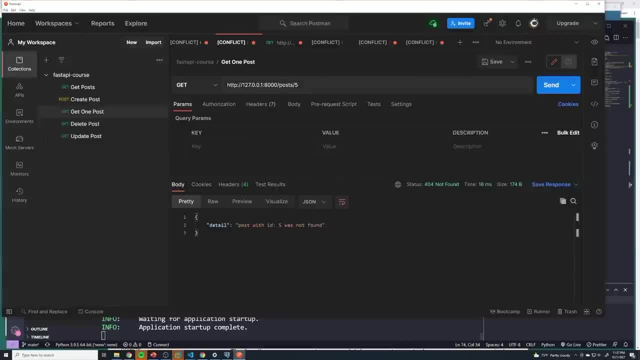 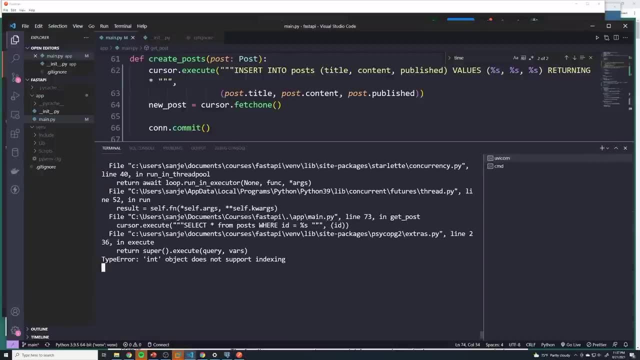 So let's see what happens when we try to run this again. I'm going to try to grab a post of 1 and let's see what happens. Alright, so it looks like we got an error. so let's take a look And it says: 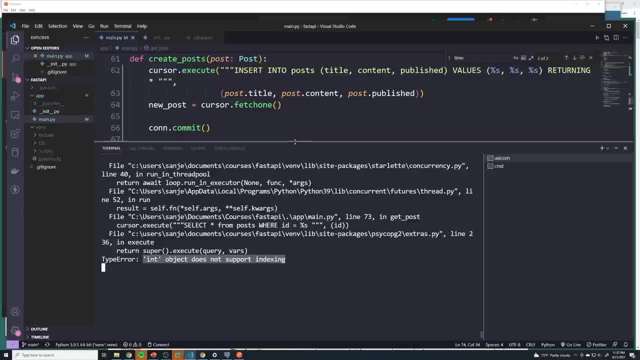 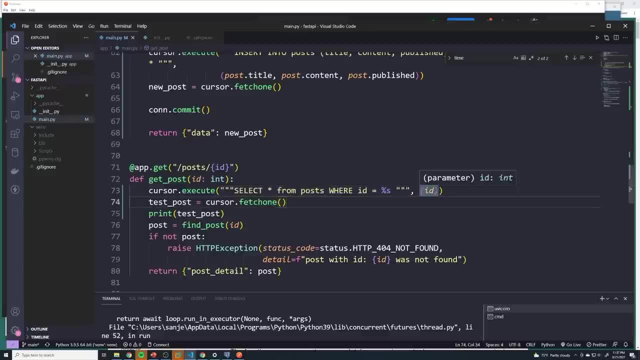 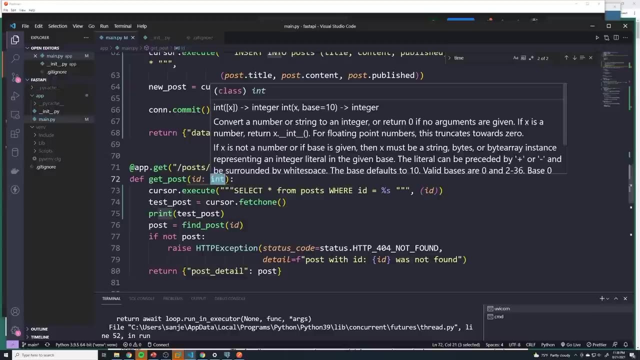 that int object does not support indexing, So it's not very helpful. However, I'll tell you exactly what's happening. Because this is a string, we need ID to be a string as well. Right now it's an integer, because we validated it as an integer and we converted it to an integer. 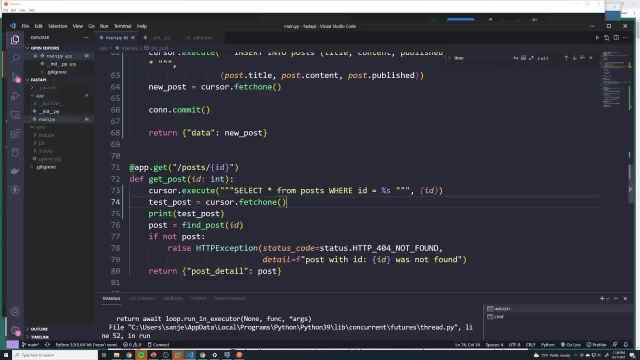 but we need this to be a string, or then it's not going to work, So we have to convert it to a string. It's pretty simple: You just do string And that's all, And at that point that should fix the issue. 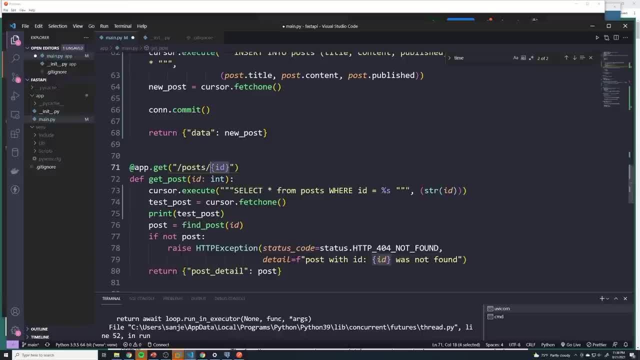 And I'm sure you guys are a little bit confused, because when it comes in as a path parameter, it's going to come in as a string. We then convert it to an int to then only convert it back into a string. And so you might think, well, maybe we should just change. 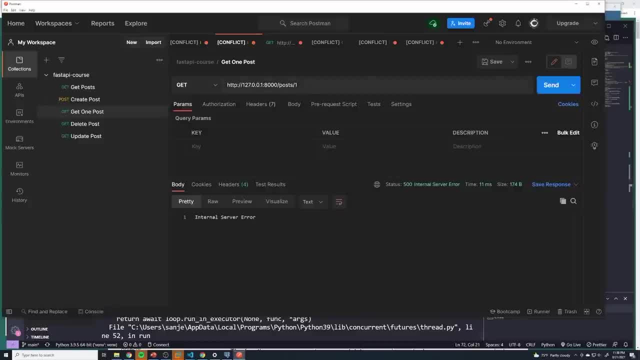 this to a string. but if you change that to a string, then it could potentially open up us to issues where the user could type in something like this, Which isn't a valid ID, So we do have to validate it as a number. convert it to an int. 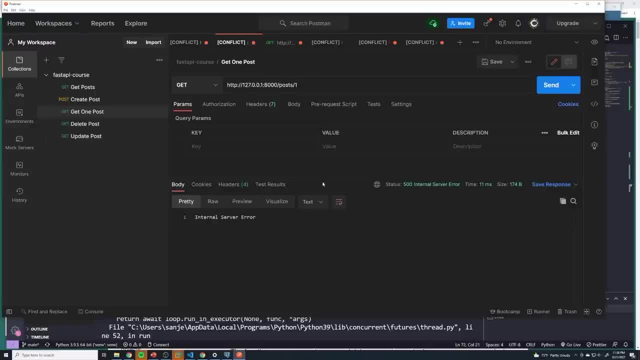 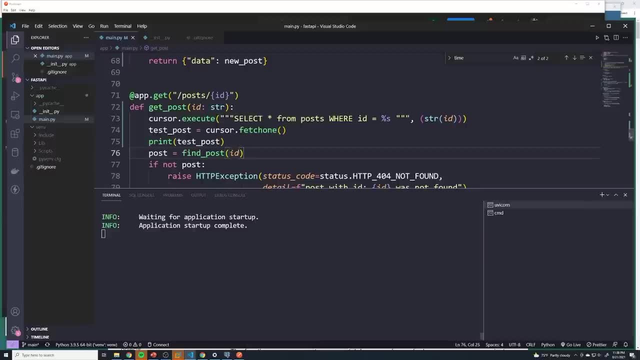 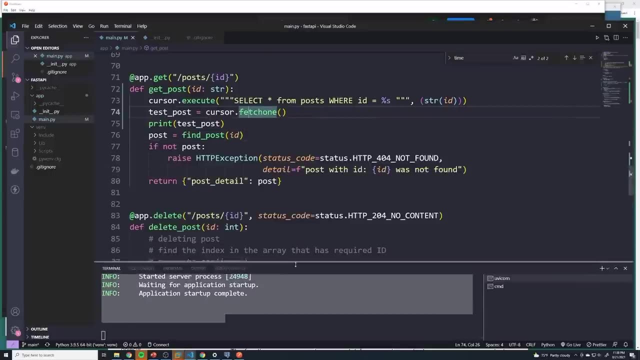 and then convert it back to a string once again. Let's save this. Our error should go away, and let's try this. Alright, no errors. so it looks like everything is good, And so now it's just a matter of cleaning up our code and getting rid of all of the other. 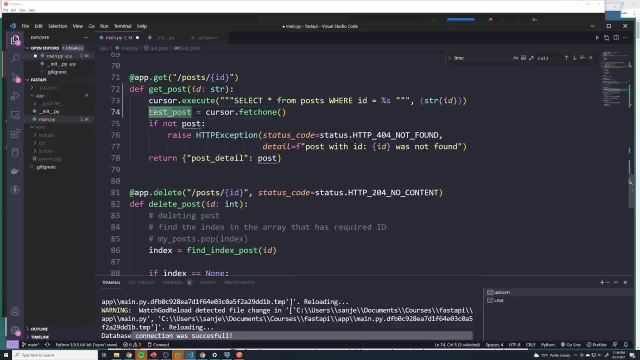 code. So I'm going to rename this. so this is just going to be post, So we can keep everything else the same. so if we didn't find a post right- which means you know the database returned nothing- it's going to be set to none and then we can raise the usual. 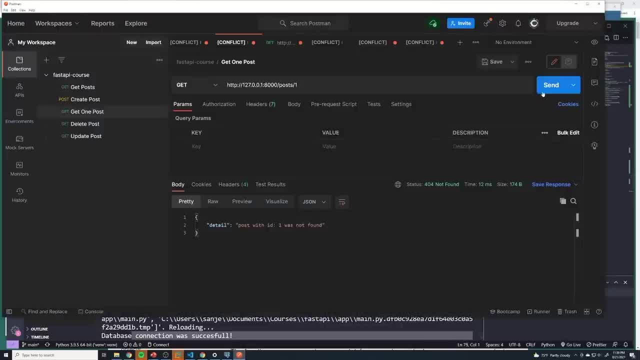 exception. but if we did find a post, we're just going to return it. Now, if I get a post of one, you can see that we've got that post, which is clearly from the Postgres database because it has the created at field. and then if I try to grab, 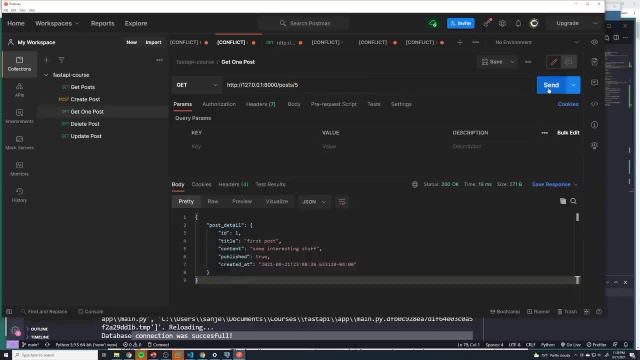 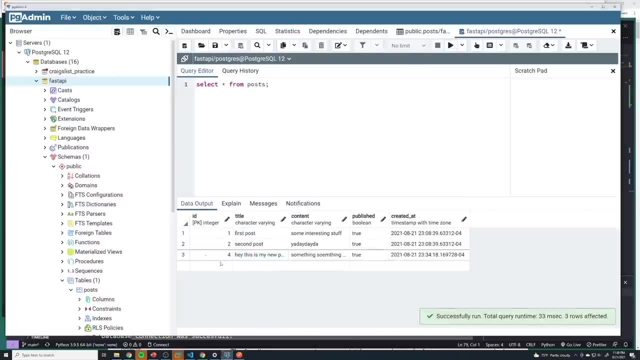 a post of an. if I try to grab the ID of a post that doesn't exist, try five- we can see that post with the ID of five was not found. and let's just double check to make sure that there is no post with an ID of five. and there isn't. 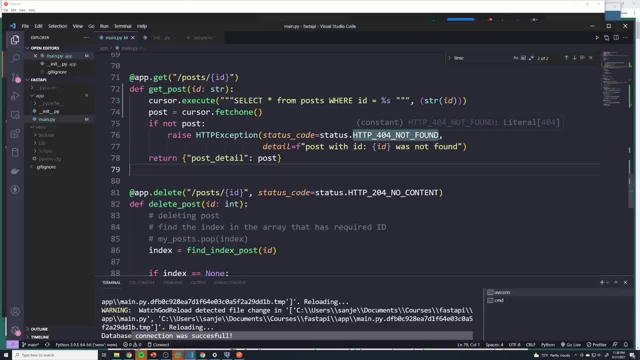 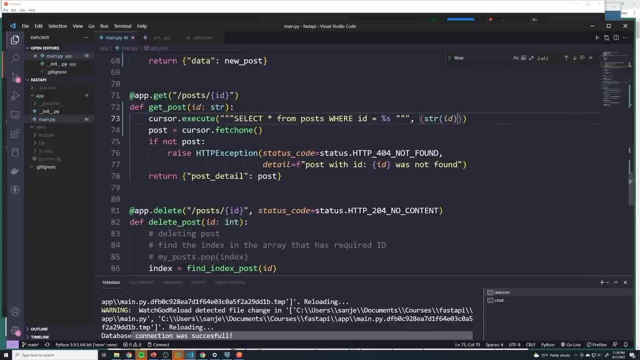 a perfect And you know, guys. one interesting thing: later down in some of the next path operations that we work on, I did run into a weird issue where, if I didn't have a comma right after this, even though there's nothing that comes after it, led to an issue. 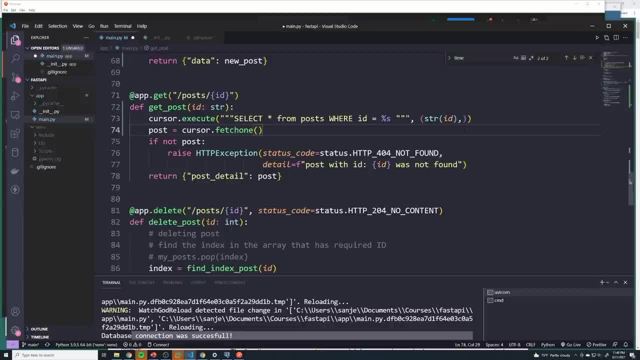 I'm not sure why it did that, but keep in mind, if you do run into some weird issues, just put in this extra comma. for some reason or another it potentially fixes some issues. So just keep that in mind. I don't have an explanation for it, you know maybe. 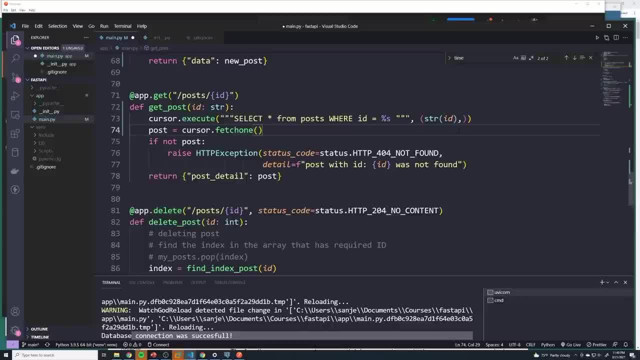 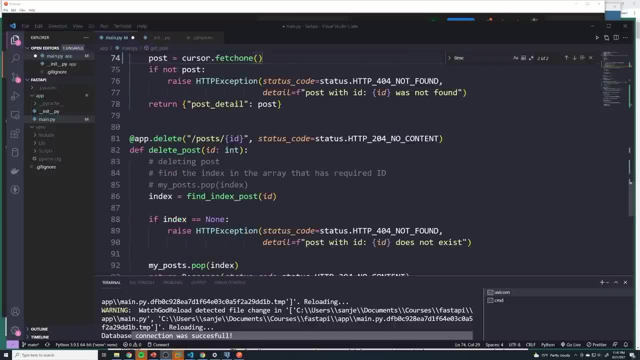 it's listed somewhere within StackOverflow, or I'm sure someone eventually or occasionally asked this question and I just couldn't find it Alright. so now let's work on deleting a post. I'm going to remove these comments to clear up some space. We're going to do cursorexecute. 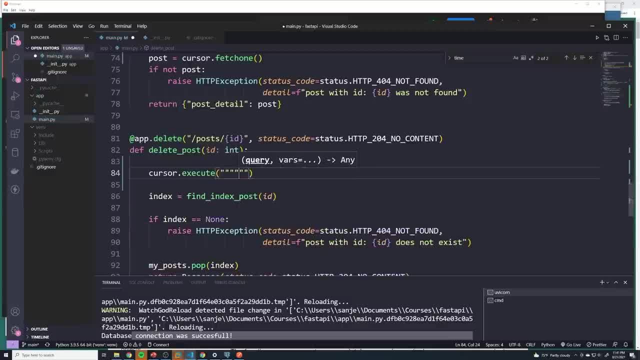 you guys should already know the exact SQL statement that we need. so it's going to be select- sorry, not select- delete from post table. and then we're going to delete by id, so we'll say where id equals and then remember, we don't want to pass in the 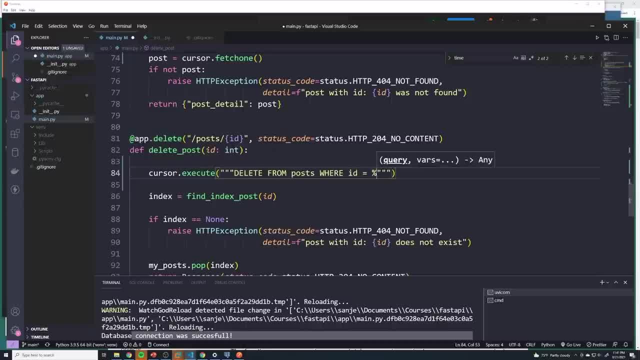 user input directly. we want to do that placeholder again and then we also want to do a returning so we'll see what that post was before it was deleted and then we'll pass in the value of the post. so this is going to be id, but we want to convert it to a string. 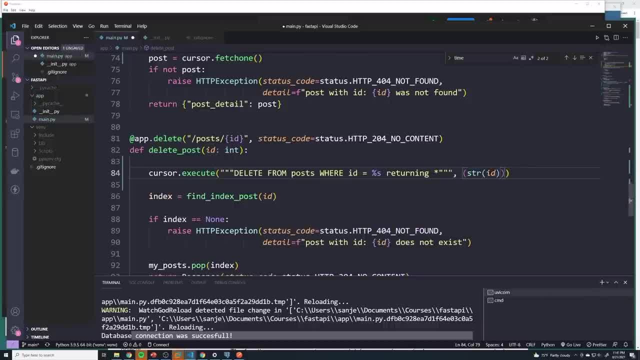 so we don't hit that error again. and then I'm going to do that empty comma just to avoid any potential issues. and then we have to do a cursorfetch1 to get the deleted post and I'm going to save this as a variable. so I'll say: 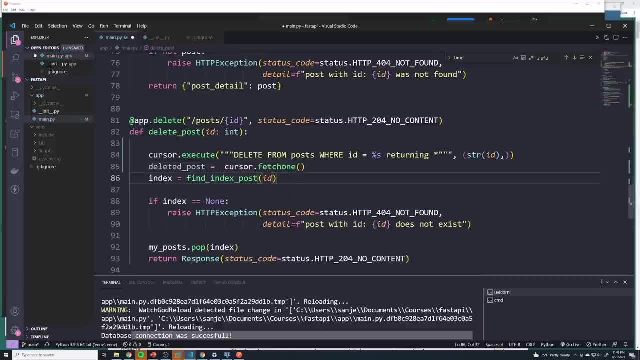 deleted underscore post equals that we can remove this. and then for this exception, when we try to grab the id of a post that doesn't exist, we can just say: if deleted underscore post, which is the post that we fetched, wasn't found, we're going to throw an error. 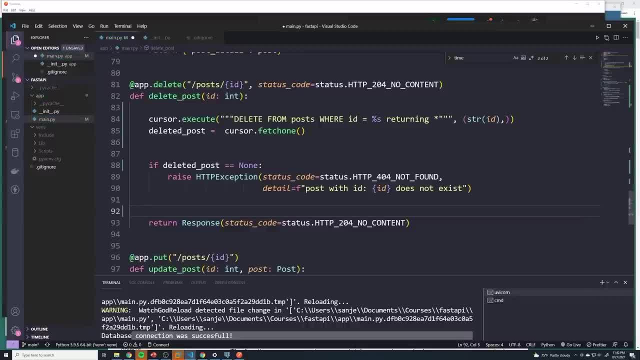 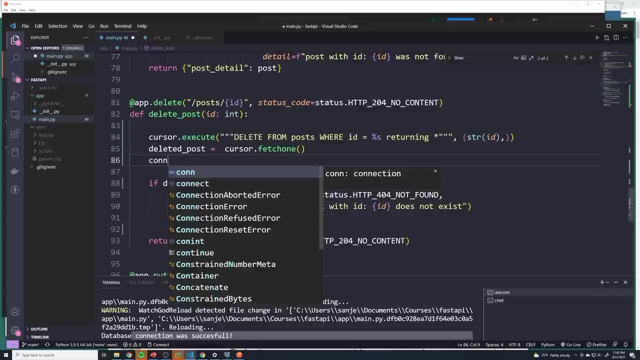 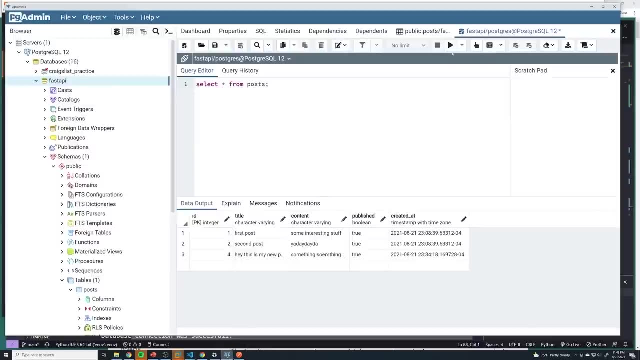 we can delete this and remember. there's one last thing: anytime we want to make a change to a database, we have to commit to it. so we'll do connectioncommit and then everything else. we can keep our code exactly the same, and then I'm just going to. 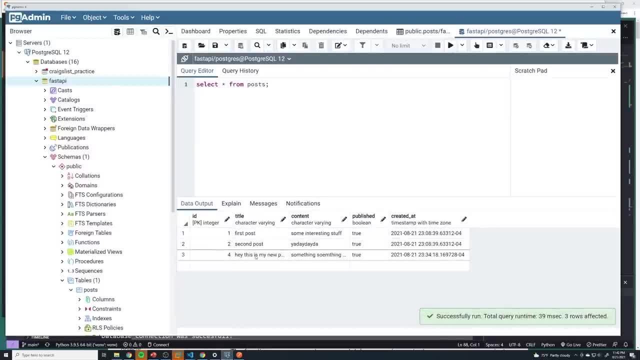 run this just to get. so we have a post with an id of 1,, 2, and 4, so let's go ahead and delete one of those. so if I delete the post with an id of 4, what do we get? oh sorry, 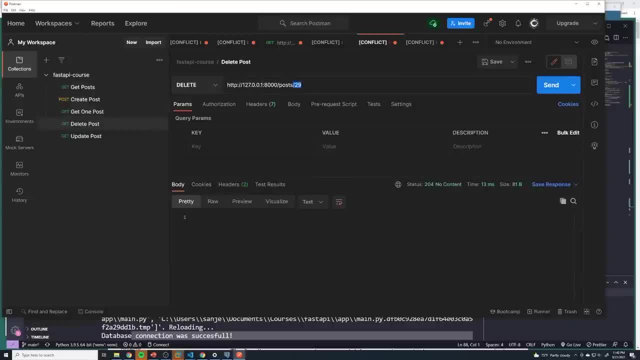 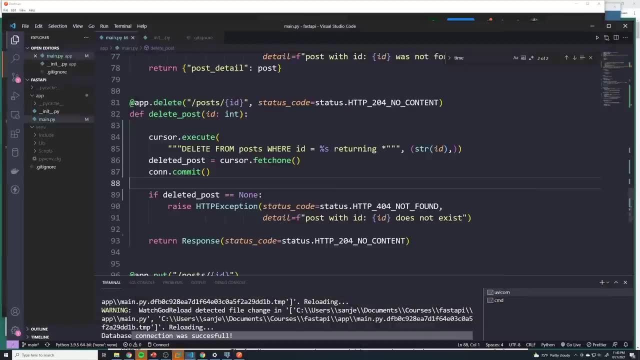 we're still under the get, let's go to our delete. this is our delete, and then we're going to delete with an id of 4 204, no content. so that's good, and let's double check our postgres database to see if it got deleted. 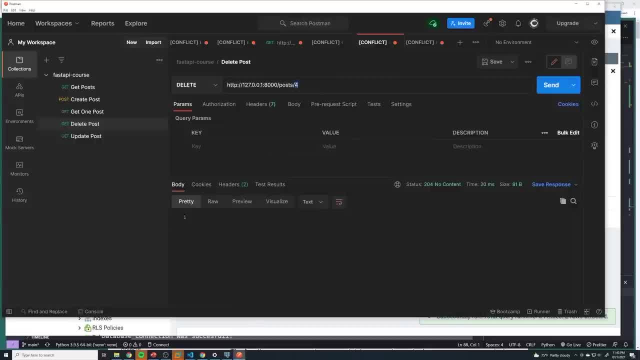 we can see that it's now gone, and then let's try to now grab the same one, let's try to delete the same post which no longer exists. we should get a 404 post with id of 4 does not exist. perfect and last but not least, the final path operation. 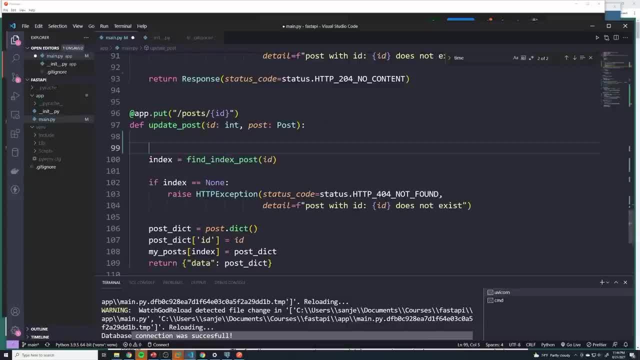 we need to update is the update post path operation. we'll grab the cursor object and we'll execute our sql statement again, and so here we'll do update posts. and then here we want to set the title. and what do we want to set our title to? well, that's going to be passed in from the user. 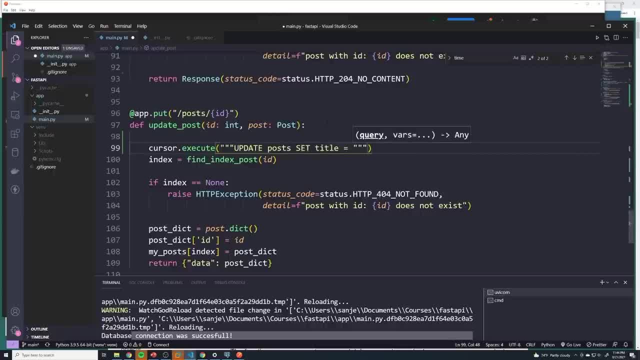 so any kind of data we get from the user, you know we have no idea if they put in you know very suspicious sql data. so we always want to put the place holders and so all the fields that they can update are going to be the title, the content. 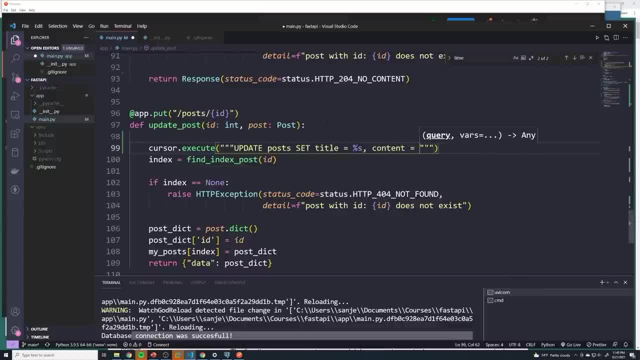 and published. so then the next one is going to be content, and the last one is going to be published and then we'll pass in those values and that's going to come from our post object. so we'll do post dot title, post dot- content and finally post dot. 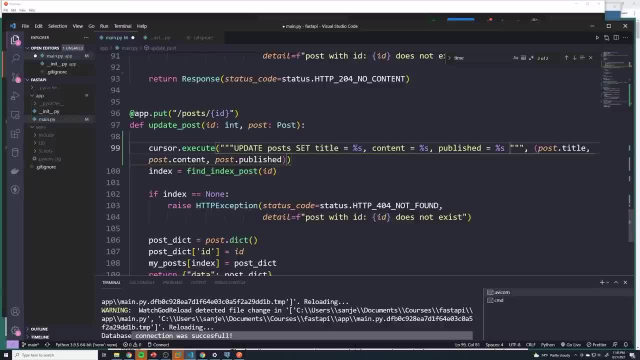 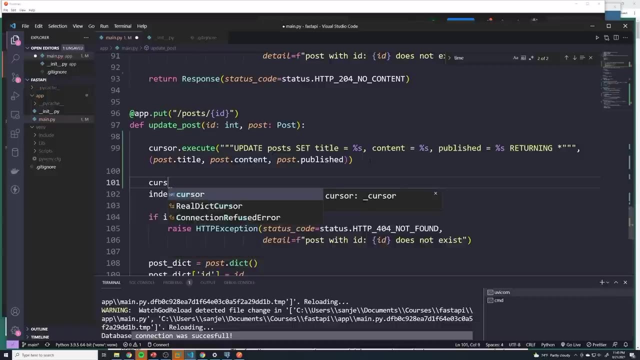 published and just like we had with inserts and delete, we can do a returning so we can actually get the returned. we can actually return the updated object, the returning star, so we can get all the columns. and then to actually fetch that updated post we have to do cursor dot. 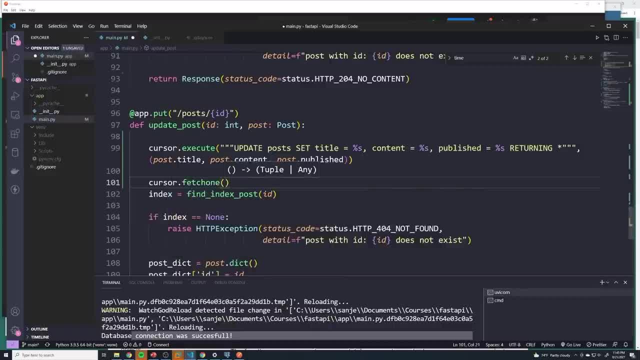 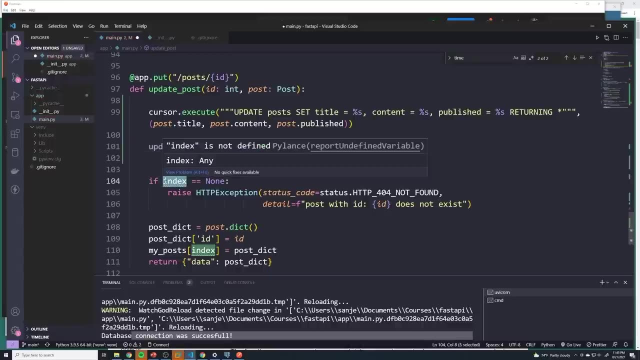 fetch one and then we'll save that in a variable called updated post and then we can remove this. this is our previous code. and then for the little check to make sure that we actually got and updated a post, we can get updated post. if we didn't, if it returned none, then we're going to send a. 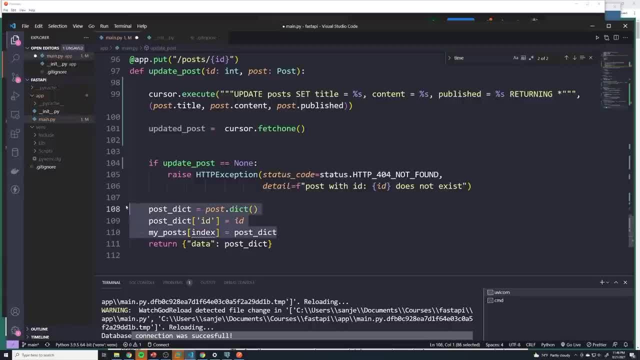 404 because a post with that id didn't exist, and then we can delete all of this nonsense and then what we return back is going to be updated post. make sure you get updated with a? d or then, if you just do update post, it tries to call it this own function, which is: 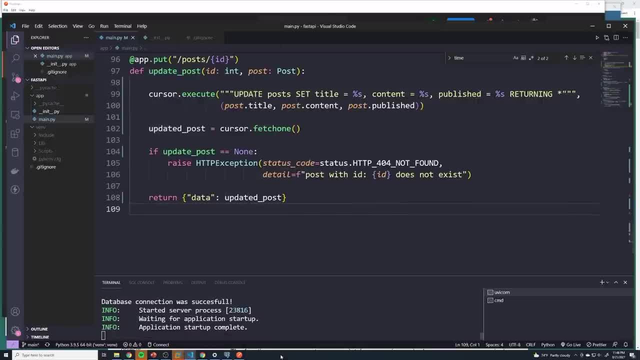 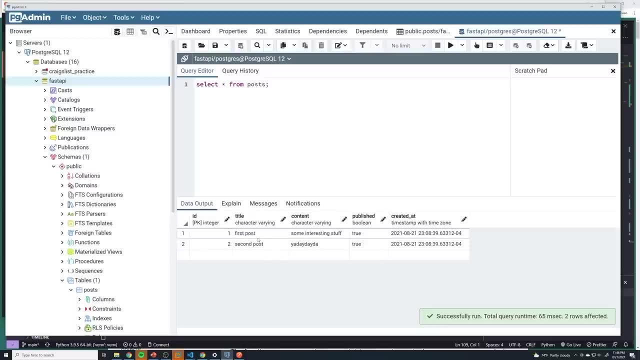 doesn't work and i'm just going to see what i have in my database. so i've got a post with an id of one, so we're going to update him. you can see. currently the title is first post. so if i go to my update post, i'm 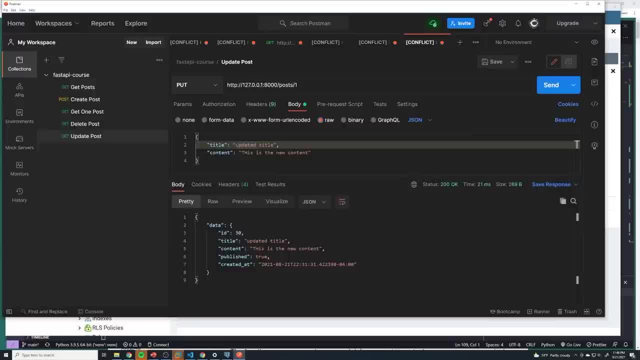 going to send it with the id of one. we're going to update that post and then it's going to have an updated title. so if we see that get updated, then we know it worked. so we'll send. do a send. we can see what we got back. 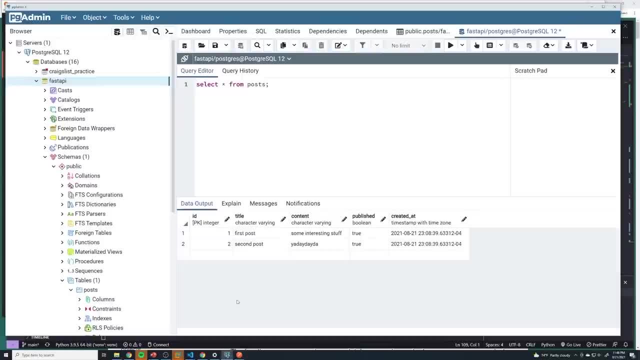 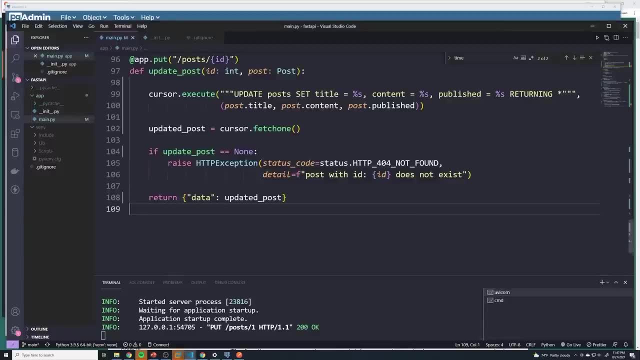 and so it looks like it updated. but let's actually double check with our database and it did not update and i'm sure you guys can take a guess as to exactly what went wrong. remember, anytime you want to make changes to a database, we need to do the connection. 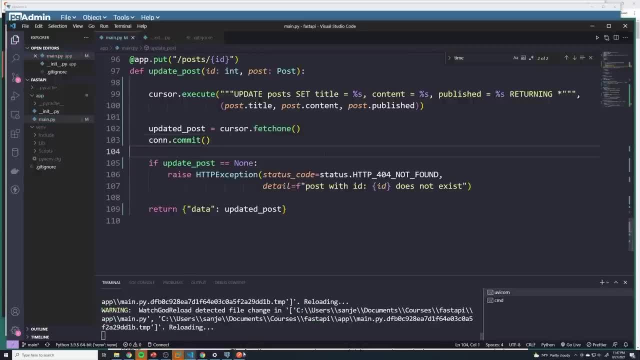 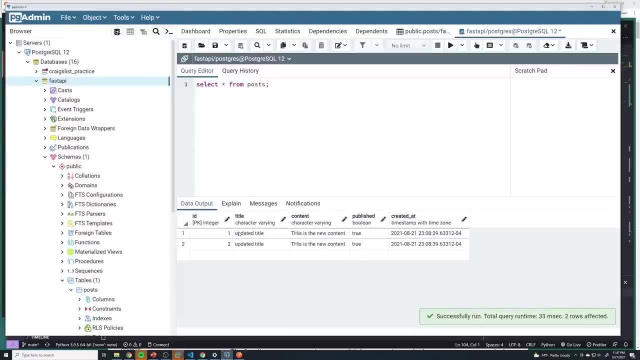 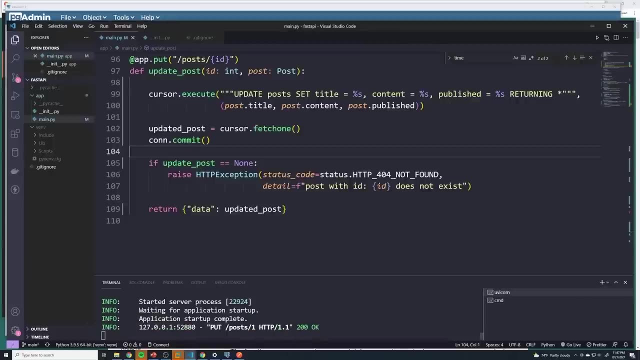 dot commit. so let's try this again. alright, so we got the same result. let's take a look at our database. run this and then we've got updated title. it looked like it updated both and, uh, that looks like a bug. so what did we do wrong? well, if you look at our 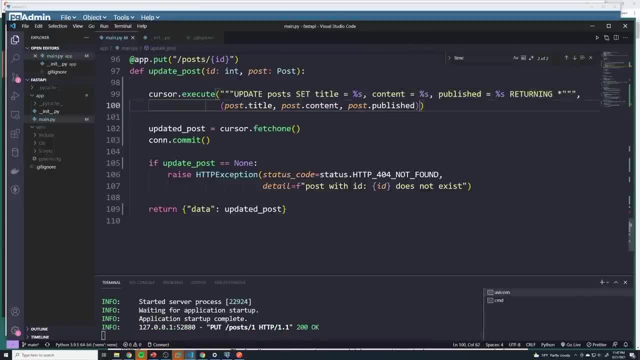 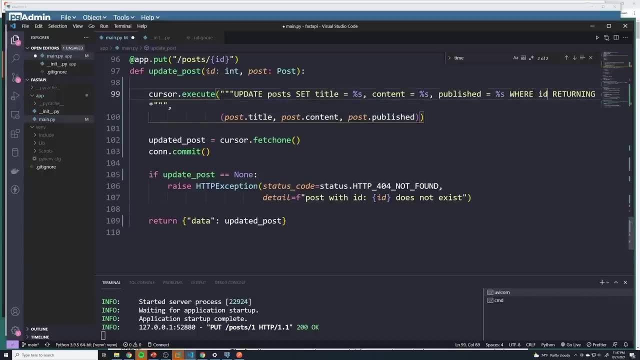 code. we're updating every single post because i didn't provide a where condition. what post do i need to update? so that's a mistake on my end. so we have to do where and then we'll say id equals and that id is going to come from this value. so we're. 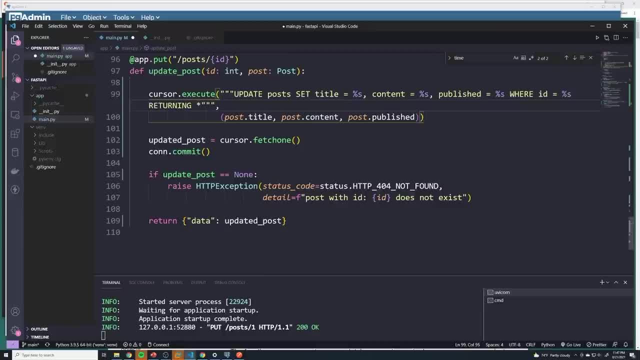 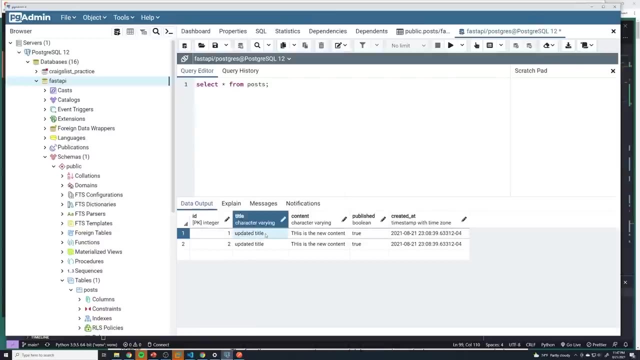 going to put another placeholder there, and then that last value is going to be the id converted to a string, just like we did before. so simple mistake. i'm going to save that and before i do that, i'm just going to change this back to first post. 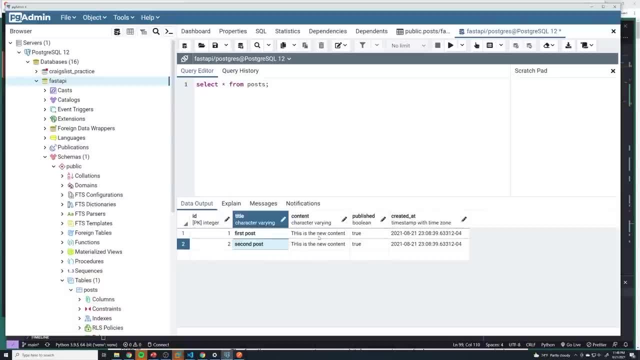 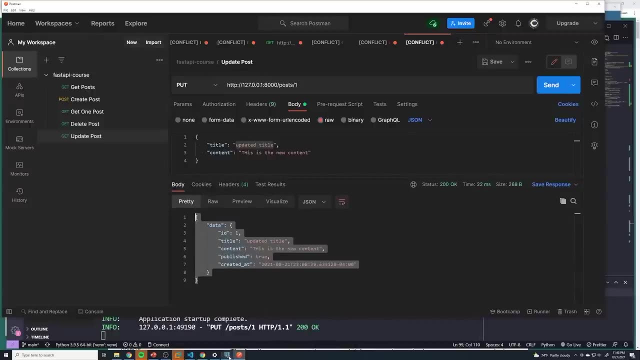 and i'm going to change this back to second post and then i'm just going to have some random text and then we'll save that. then let's update this. alright, so we updated our code and then let's take a look at our database. we'll run it. 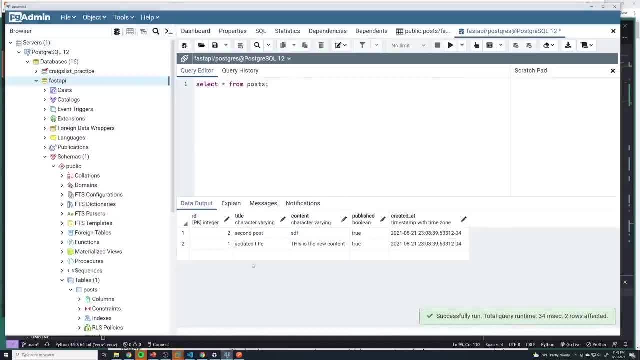 run this again and we can see that it was updated, and you'll notice how that first post then moved down the list because it was most recently updated. but we updated just one post this time. and then, last but not least, let's try to update a post that doesn't exist. 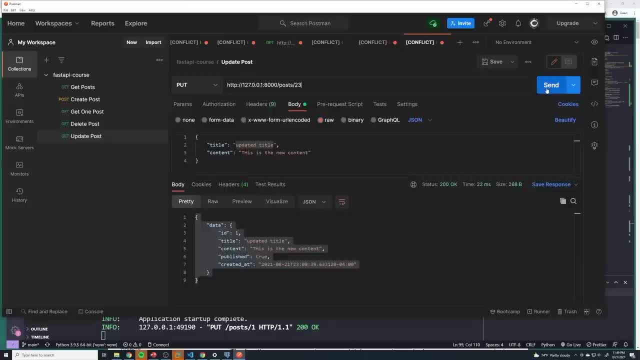 so i'm going to search for an id of 23, try to update that and then, if i do that, we can see that we get a little bit of an error. so what happened here? we got data equals null, and so it looks like this didn't work. 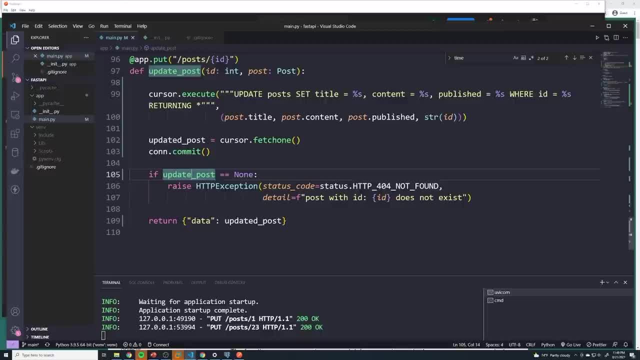 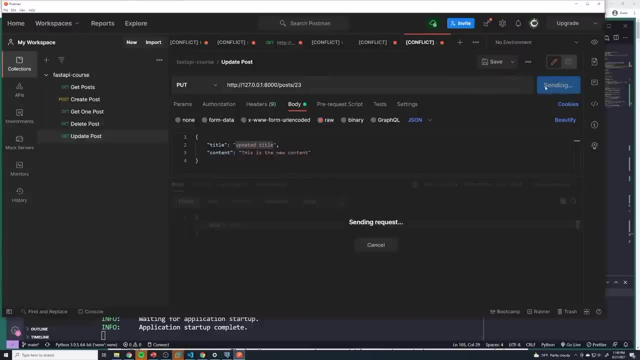 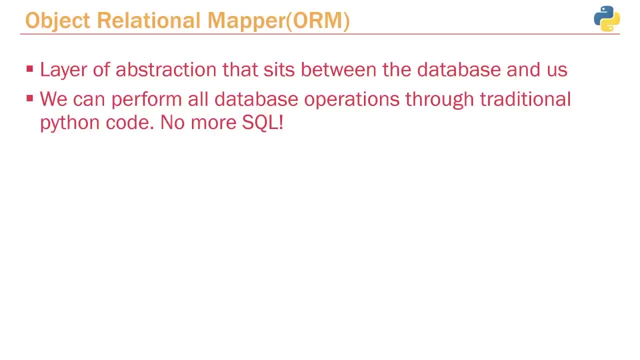 and it looks like it changed back to update post, so make sure you reference this variable. so i need that d now. let's try that. and now we get the correct 404 when it comes to working with a database within a python application, or really any application. 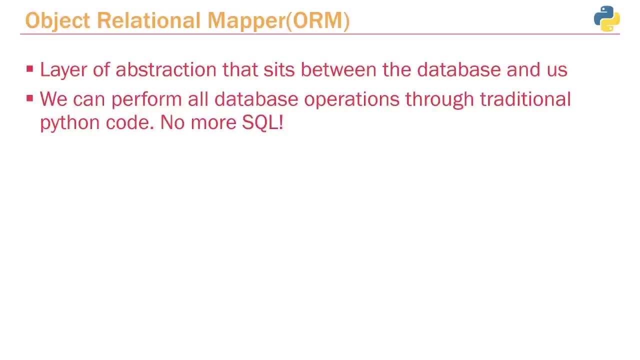 across any language. there's a couple of different ways of interacting with the database, and so we saw how we can use the default postgres driver to talk to a postgres database by sending sql commands, and this is my preferred method of working with databases because i'm fairly comfortable with sql. 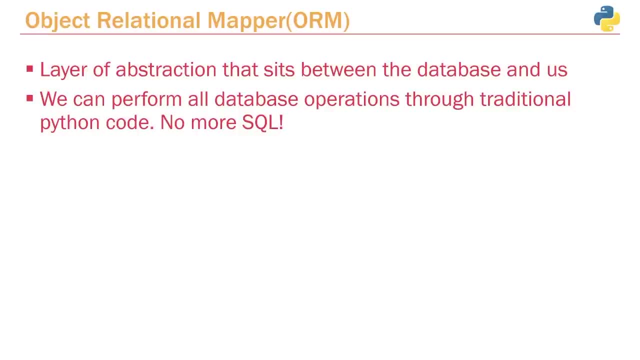 and so it just makes sense to use raw sql and send that directly to postgres, using whatever the default postgres driver is for your specific programming language. however, there are other methods, and so you'll see that one of the popular ways of you know, really working with databases. 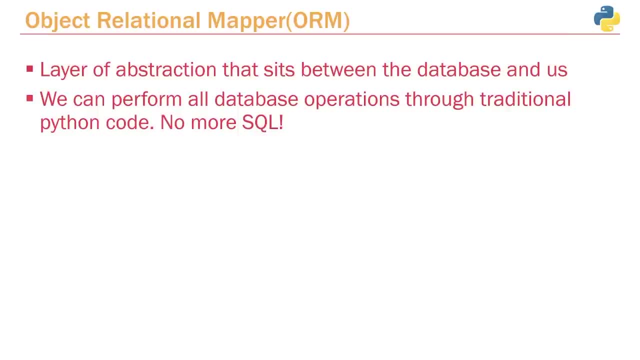 is using what's referred to as a object relational mapper or an orm, and so an orm is a layer of structure that sits between the database and our fast api application, and so we never actually talk directly to a database anymore. instead, we talk to the orm, and then the orm will actually 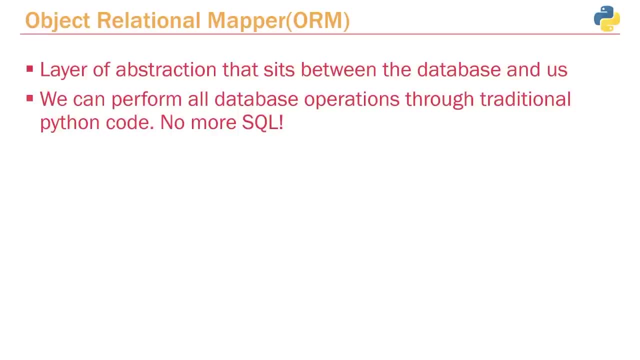 talk to our database, and so some of the benefits are is that we don't actually have to work with sql anymore. so, instead of using raw sql, what we'll do is we'll actually use standard python code calling various functions and methods that ultimately translate into sql themselves. 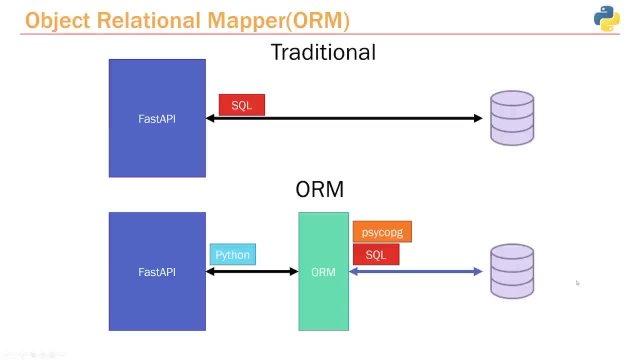 so let's see what that actually looks like. and so, with our traditional application, which is what we have now, we've got our fast api server and it's going to talk to our database by sending sql using the default postgres database driver. however, with an orm, what we can do is 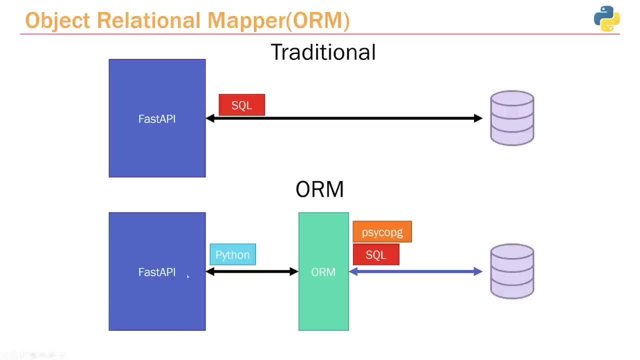 fast api no longer has to talk sql. instead, fast api will actually use regular python code to send- you know- specific commands to an orm and then the orm will take that python code, convert it into regular sql and then, using the same database driver that we're using for it'll actually talk to. 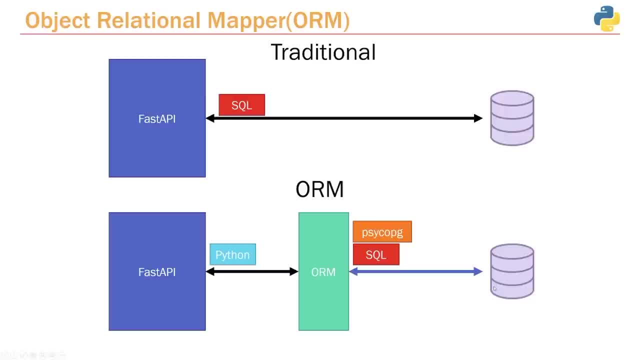 the database and then it'll eventually send that result back to us, because the databases they can only talk sql. however, by doing like this we can kind of abstract away that sql complexity and make use of very common python objects and various other python features to actually generate and build queries as 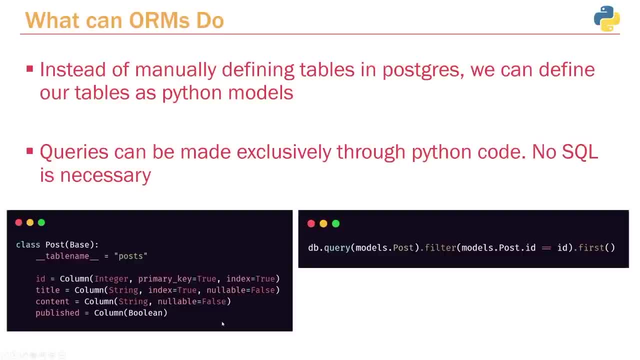 well as to create and define tables. so let's take a look at what an orm ultimately allows us to do. so one of the first things is, instead of us going into you know, pg admin and creating the tables and all the columns ourselves, what we can do. 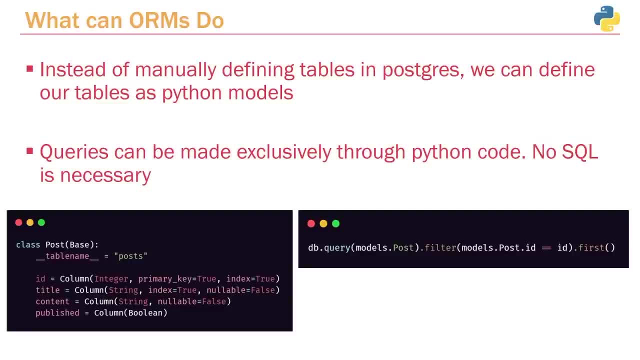 is, we can define our tables as python models, and so if you take a look at the code down here, what we can do is we can actually define what our tables in postgres are going to look like, and so you can see here, we give it the table a name and then we can specify. 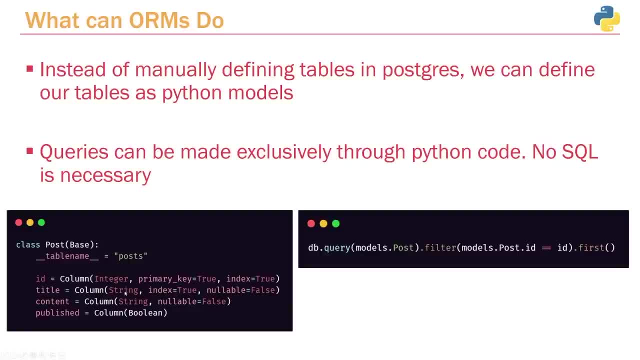 each of the columns you'll see a lot of the common fields that we already worked with. so the type: so this is an integer, this is a string. we can also see if a field is nullable. we can see that the id is set to be a primary. 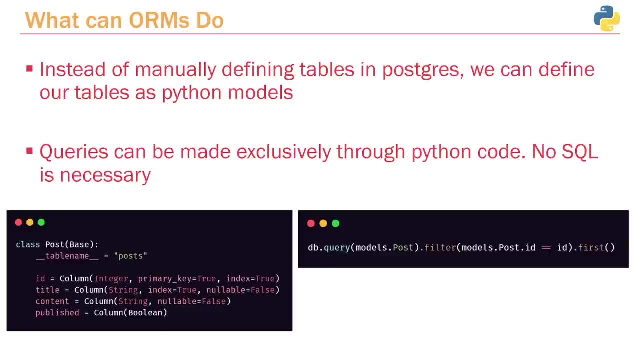 key. so we're using standard python classes to define our tables, so that we don't need to do it ourselves using pgadmin, and on top of that queries can be made using regular python code so we can actually chain on different methods to construct various python to construct various. 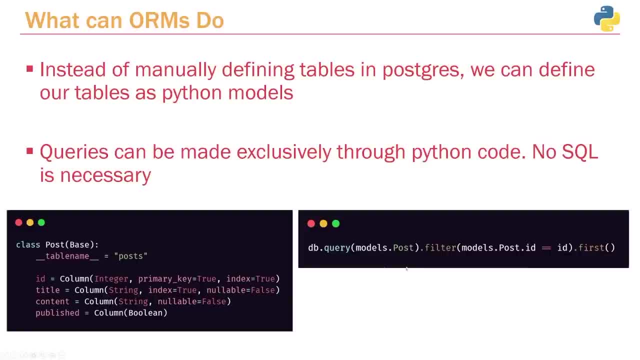 sql queries and so if you take a look at one of the queries down here below that i provide as an example, you can see we just do query, we provide the specific table that we want to query and that's going to be based off of the specific models, and then we can just pass. 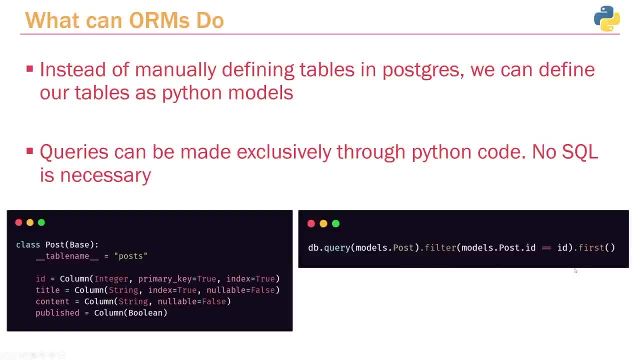 in whatever filter commands and then grab the first entry so you can see that there's no sql anymore, it's just standard python code, and so that makes it a little bit easier for some people who may not be as strong on sql, and so they don't have to worry about. 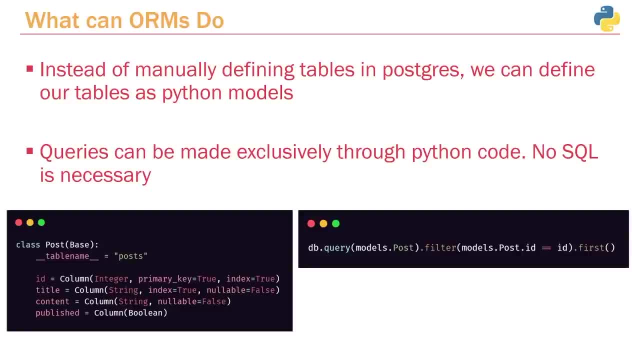 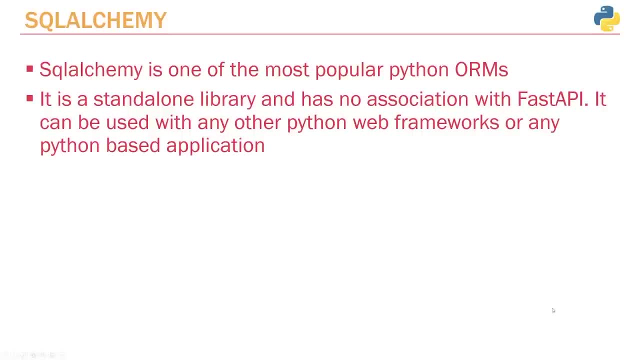 writing these complex sql commands. they can just chain on specific methods to a db query to generate their final sql commands, and so the you know there's a couple of different orms. i'd say the most popular one within the python world is sql alchemy, and one of the things to keep in mind. 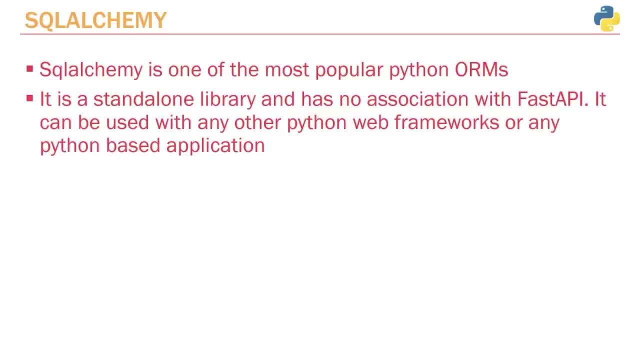 is that this is a orm, that's a standalone library, right? so this has this library has nothing to do with fast api. we're going to use it in our fast api application, but i want you guys to understand that it actually has no relationship with fast api. 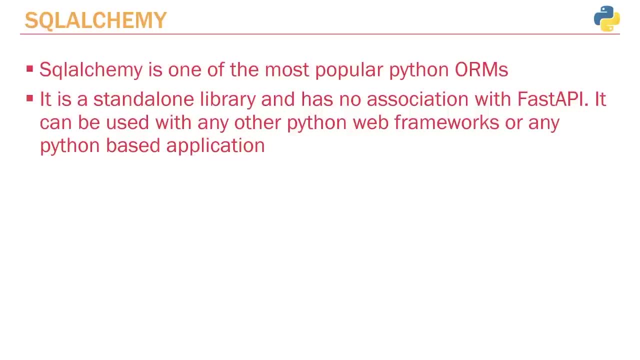 it's not part of fast api. it's its own library and you can use sql alchemy with any web development framework. you can use it with any python application, even if it's not a web application as well. so in the next video we'll start taking a look at how to work with sql. 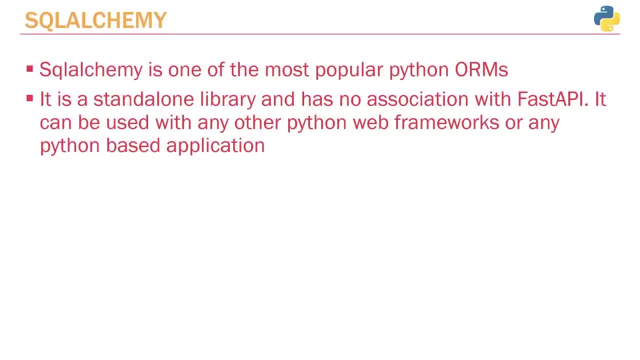 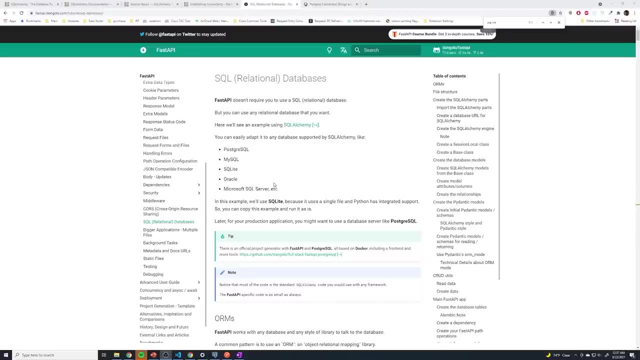 alchemy and how to set up a database connection using sql alchemy instead of using the default postgres driver. okay, so in this lesson we're going to start taking a look at sql alchemy and get that set up in our project, and so there's a couple of things that i want you guys to take. 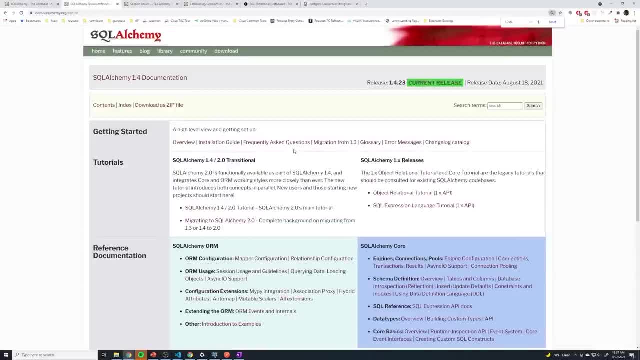 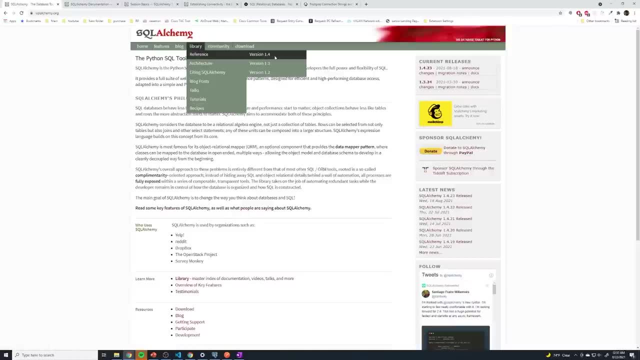 a look at. so the first thing is i want you to go to the sql page, so if you just search for sql, you'll get to the main page. and then, if you want, to go to library, and then references and then version 1.4, which is the one we're going to use. however, 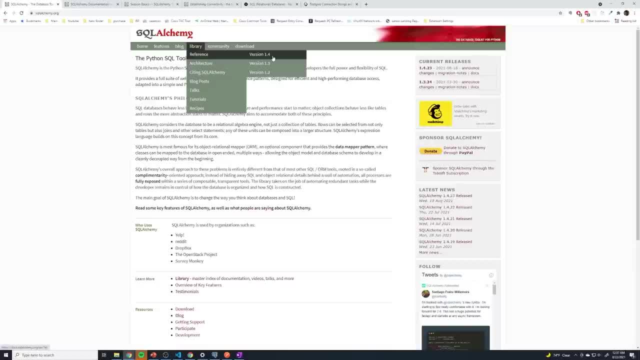 i believe they're going to come out with a version 2.0, which is going to be pretty different. so if you are watching this video in the future, you definitely want to install version 1.4 so that you can follow along with this course. 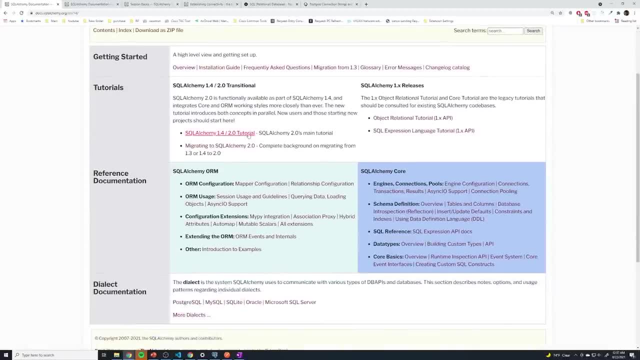 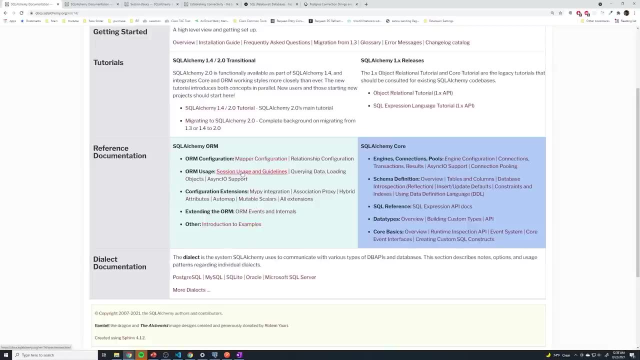 so you can click on that, and so there's a nice little tutorial you can follow, and then there's also some reference documentation when it comes to setting up the ORM. so if you click on session usage, this will show you how to set up a session. however, if you go to the 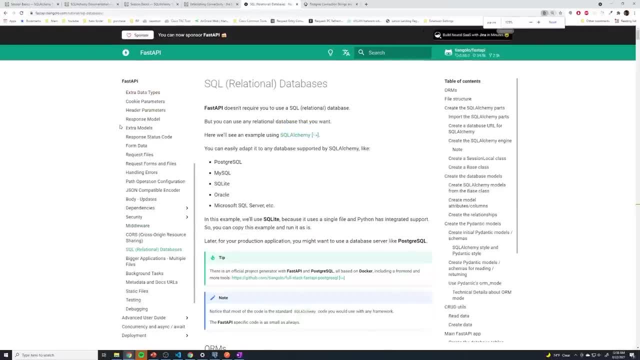 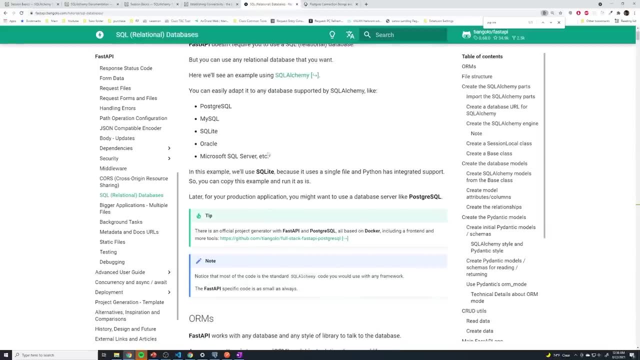 fast api documentation as well. fast api- they've got great documentation. so if you go to the documentation and then select sql relational databases, this is going to show you how to set it up with sql alchemy. so first things first, let's go ahead and do a pip install for sql alchemy. 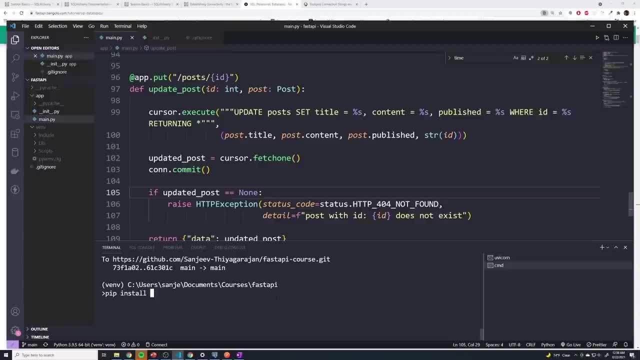 so we'll do pip install and then sql alchemy. now, guys, i want you to remember that. well, first of all, i'm running 1.4.2.3, but the thing is, sql alchemy doesn't know how to talk to a database. right, it has all the code for us. 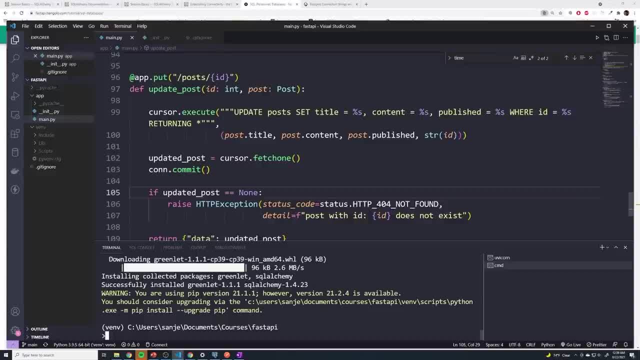 to write python, define all the models and things like that, but it doesn't actually know how to talk to a database. it only needs a database driver. and so if you take a look at all of the packages that we already installed by doing a pip freeze, right, we in the last video or in the last section. 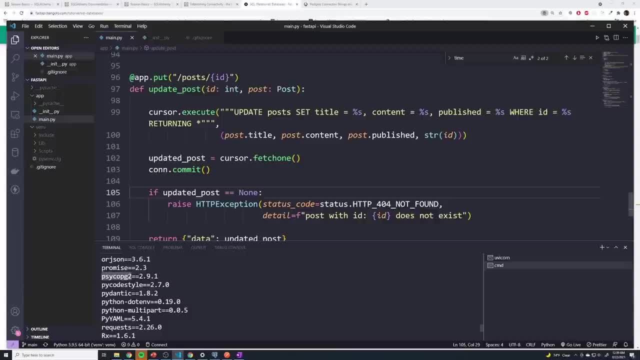 we installed our postgres database driver, so whatever database you guys plan to use. so if you want to use a mysql database with sql alchemy, you have to make sure that you install the underlying driver as well, because ultimately that's what's used to talk to the database. 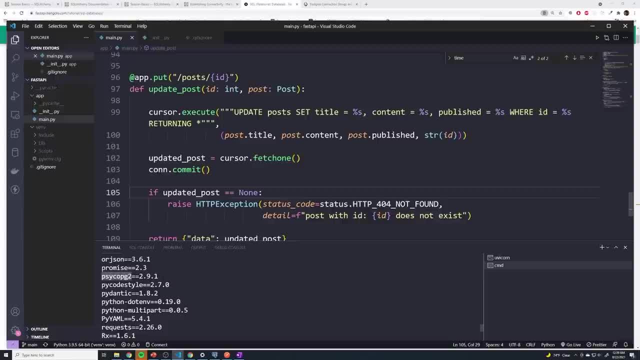 since we're using postgres, we need to install this as well, but since we were using it originally in the previous sections, we had it. we already have it installed, so we don't need to worry about doing that, but keep that in mind. sql has no way to talk to a database. 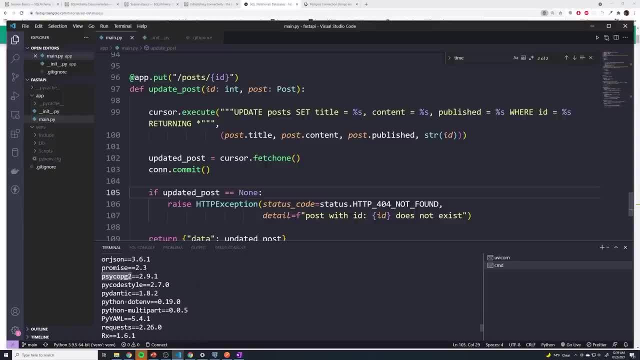 it still needs the underlying driver to communicate with it, and that's usually how all ORMs work. but now that we have that inside our app folder, I'm going to create a new file and I'm going to call this databasepy. so this is going to handle. 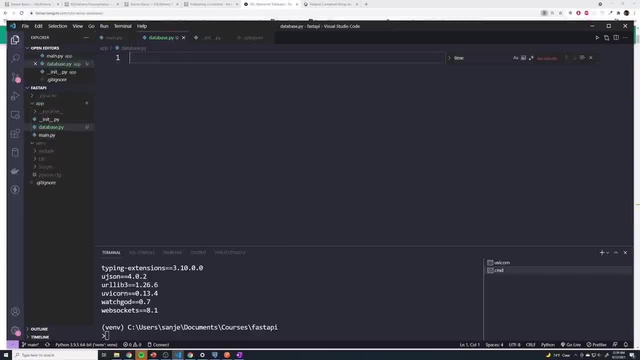 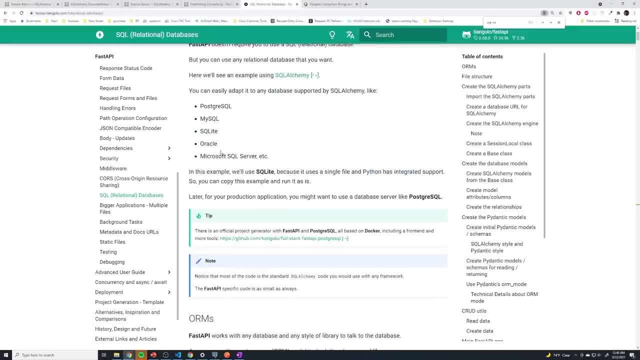 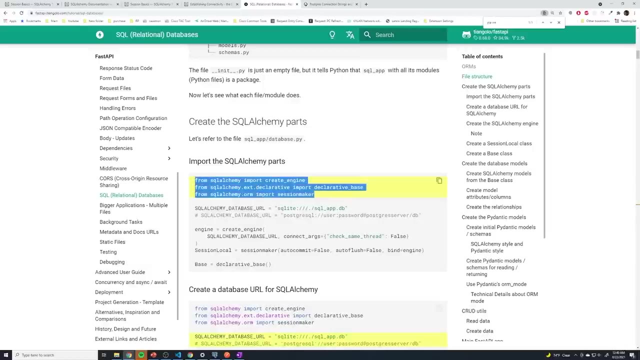 our database connection and from here what I'm essentially going to do is just really follow this documentation. so if you take a look at it right here, we can just copy all of this code right here when it comes to importing statements. so this is just going to import all of. 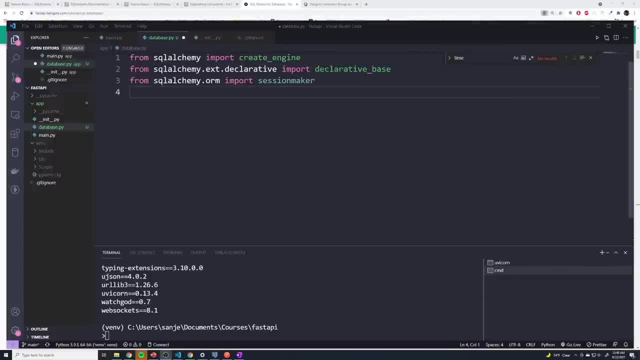 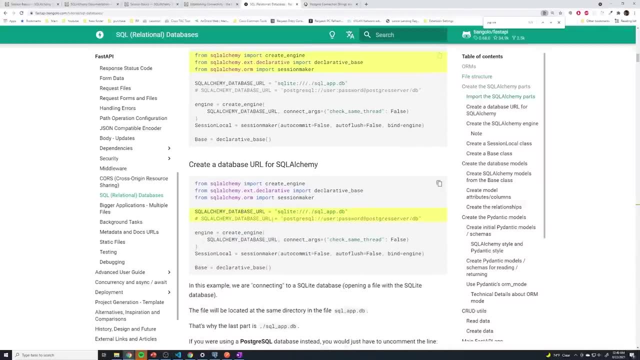 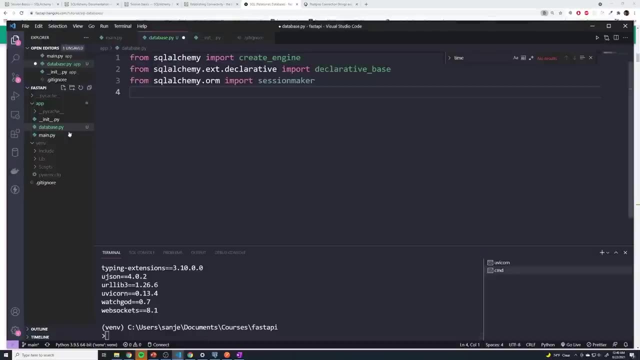 this sql alchemy code that we want, alright, and then we have to specify our connection string. so where is our postgres database located? and so, if you take a look at how we had this setup before using the default postgres database driver, right, we passed it into this connect function. 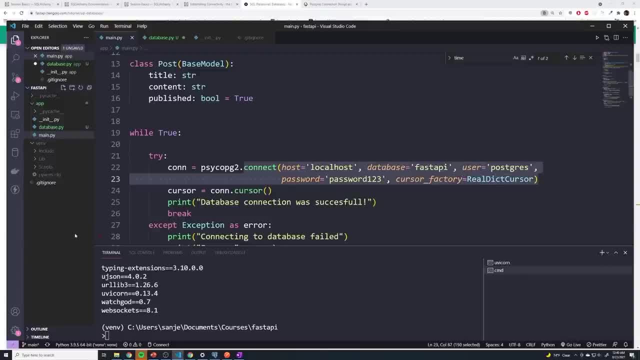 however, a lot of times when it comes to working with databases, there's a unique url that you create to connect to any kind of database and there's a specific format for that, and the format for that is actually pretty simple. so go to databasepy and then I'm going to. 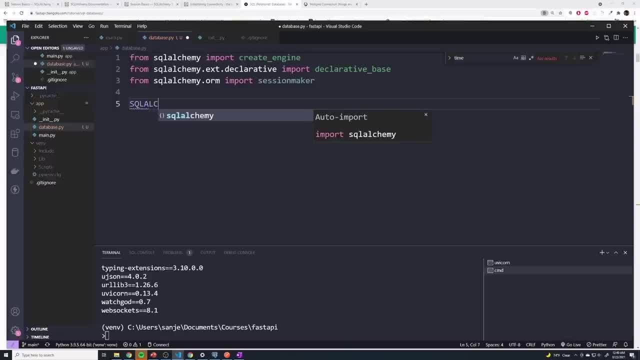 create a variable called sql alchemy, underscore database, underscore url. so this is going to be a regular string and the structure of the url for postgres database is going to be postgresql, because that's the type of database colon: slash, slash. then we have the username that you have to put in. 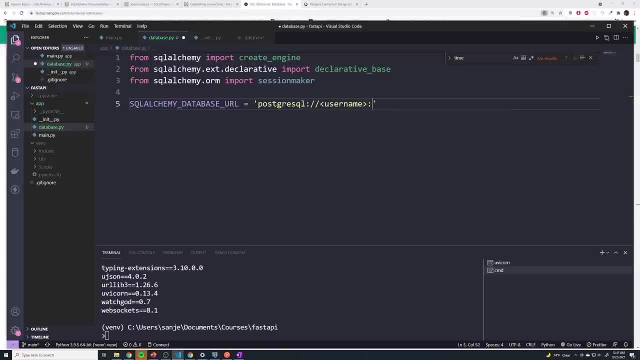 colon. then we have the password and then we do at and then this is going to be the ip address. i'll say ip dash address, slash host name. whichever one you're using, in our case that's going to be localhost. and then you have to provide the database. 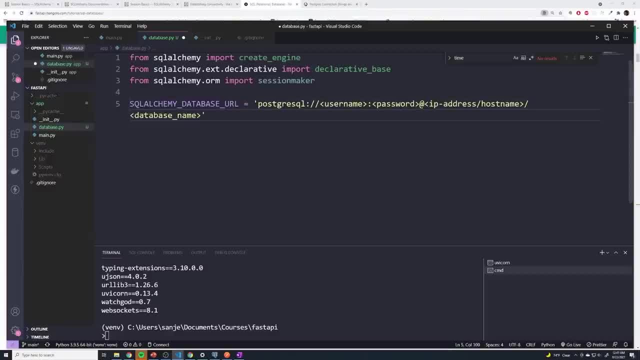 name that you want to connect to. so that's the format of a connection string that we have to pass into sql alchemy. and then what we do is we say we have to create a engine. so the engine is what's responsible for sql alchemy to connect to a postgres. 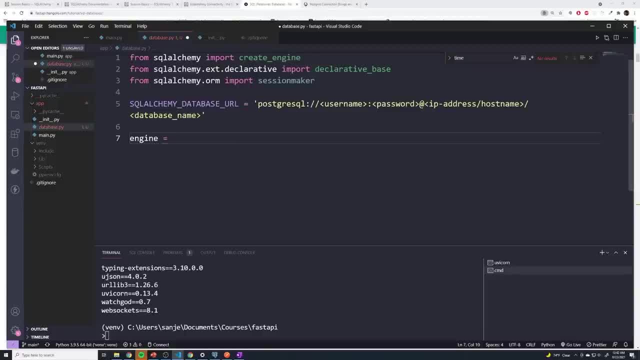 database. so you do engine equals, and then we're going to reference this- create engine- and then we pass in our connection string, so we'll say sql, alchemy database url. however, this is not filled in yet, so we're going to fill in this data, so go. 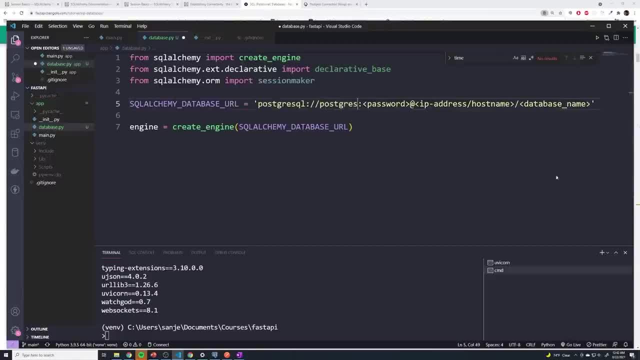 ahead and put in your username. so if you haven't created a custom user, it's going to default to postgres. put in your password. so we'll do password 123 for me. the ip address, slash host name: this is going to be localhost. and then the database name: this is going to 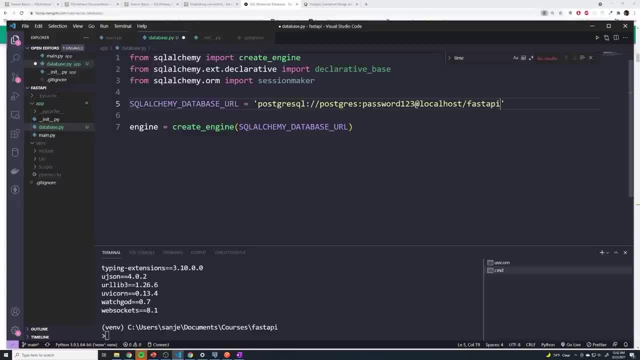 be fast api or whatever you created your database as. so that's your connection string and, like i mentioned before, it's never good to hard code this value somewhere in your code, because now you've got your password stored in your code and it's going to get checked into github and then anyone 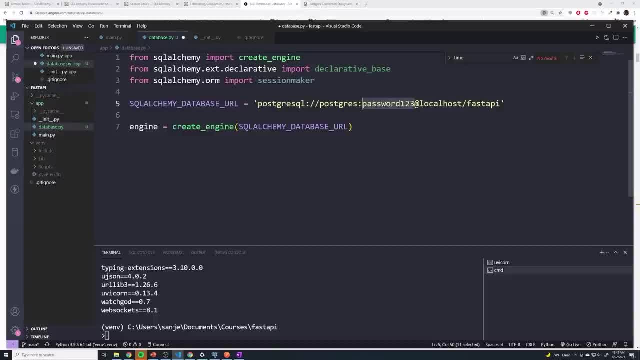 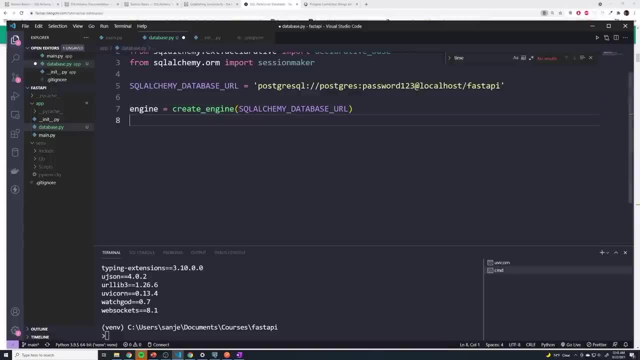 can see it, so this is bad practice. however, we will change this in the future, right? so, like i said, the engine is responsible for establishing that connection. however, when you actually want to talk to the sql database, we have to make use of a session, so we do a. 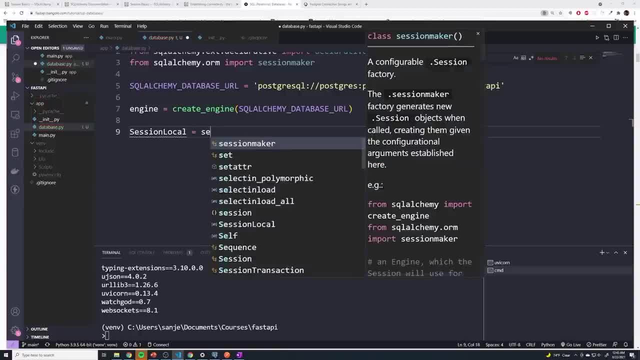 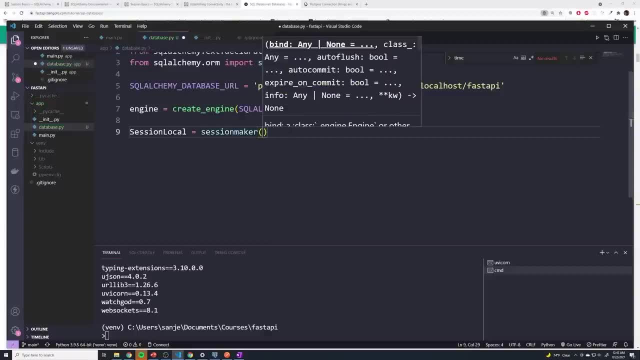 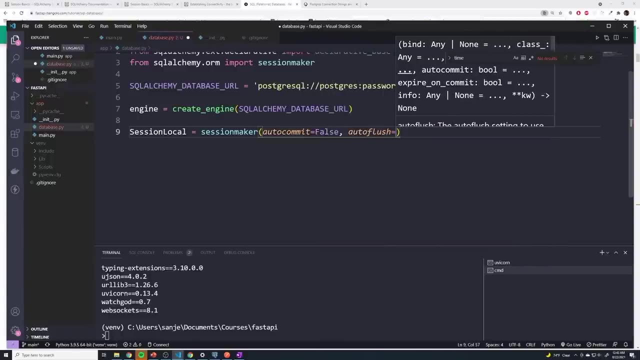 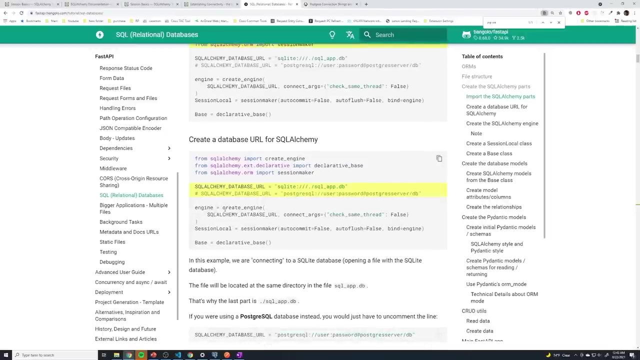 session local equals session maker. and then we just pass in a couple values, so auto commit false, auto flush equals false, and then bind equals engine alright, and all of these values. these are just some default values. now keep in mind when you are creating the, when you use. 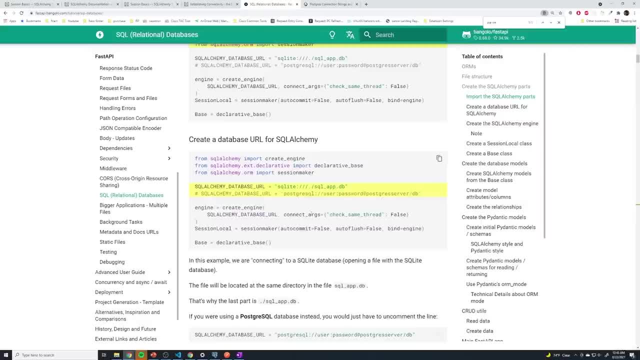 the create engine function. if you are using a sqlite database, you have to pass in this option as the second parameter. so you do the database url and then you do connection: args equals check. same thread equals false. this is something that is exclusive to sqlite, because i guess it's just running in memory. you don't need. 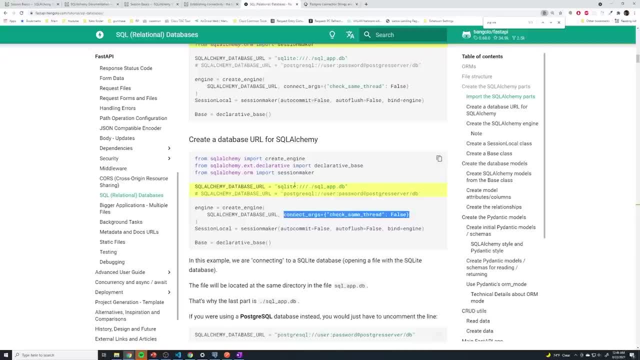 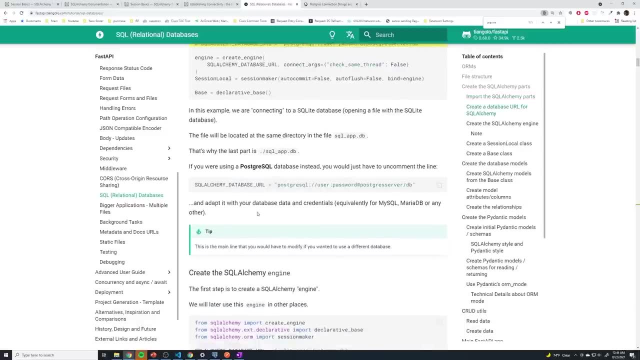 to do this for postgres. you don't need to do it for any other sql based database, and then you can see in the documentation. this is what the connection string will look like. so if you are using a sql based database, you can just use the sql sql. 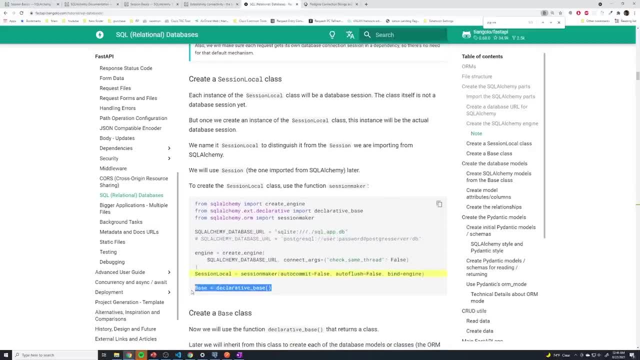 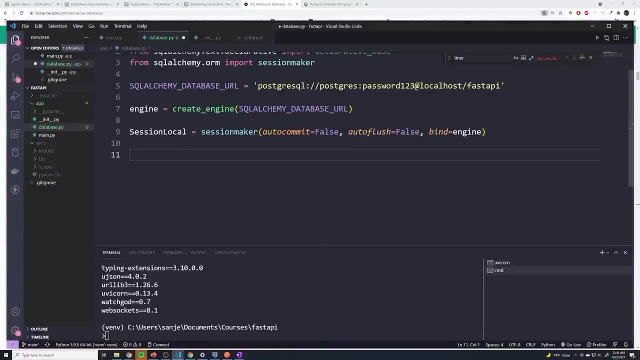 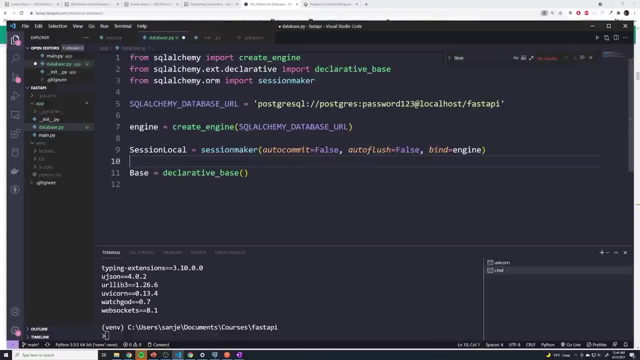 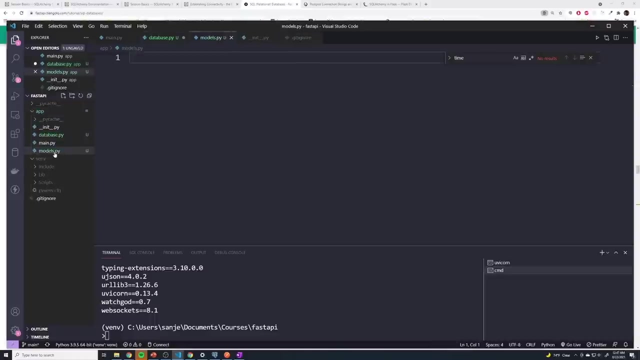 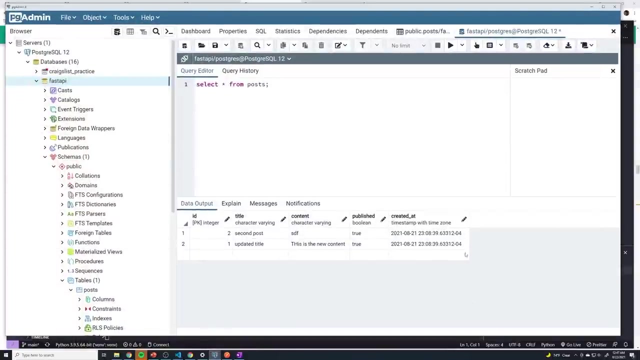 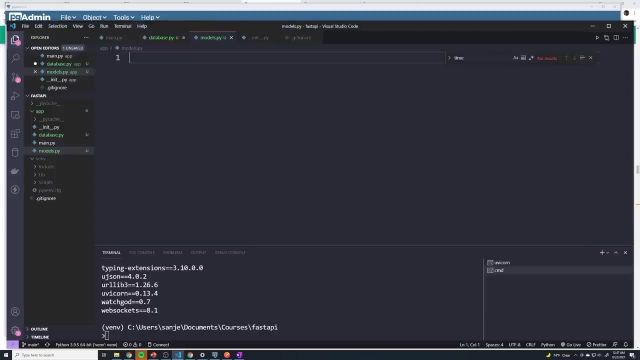 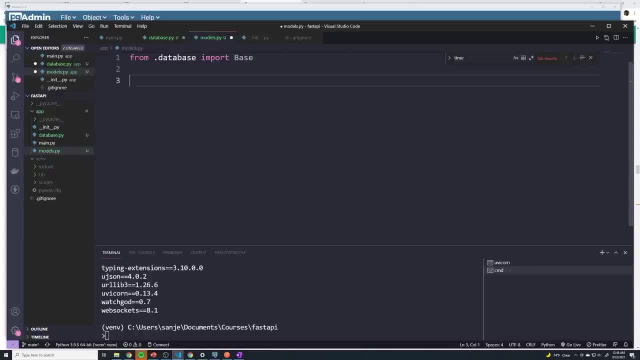 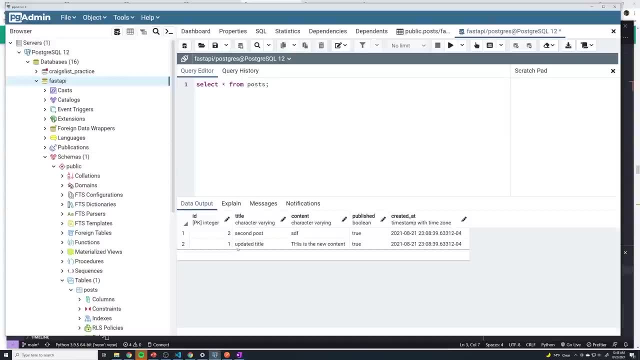 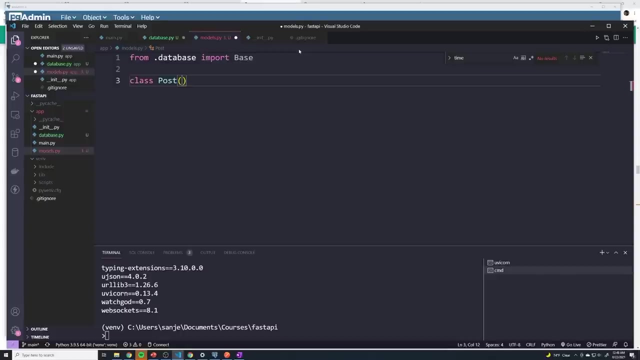 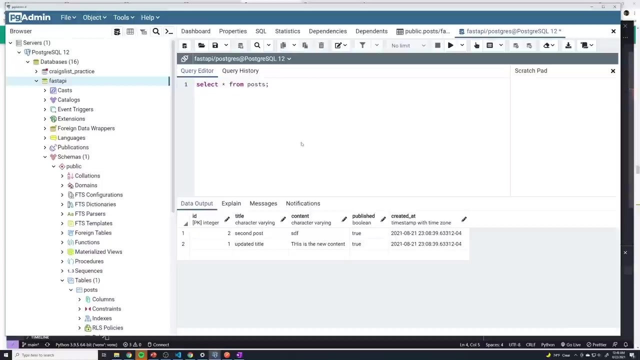 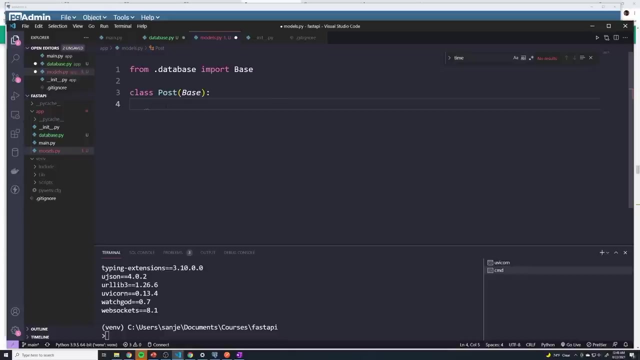 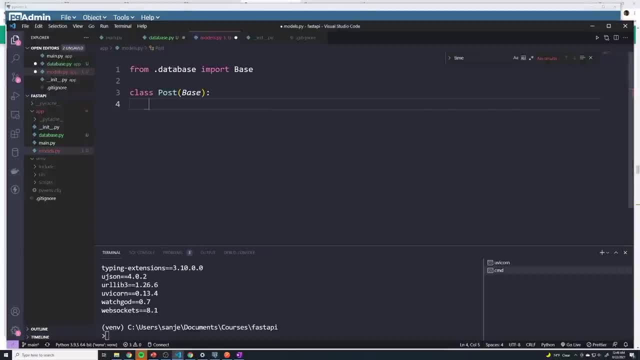 name right now is called posts, So I think we should just keep it at that, So we could say: underscore, underscore- table name, underscore, underscore, equals and then the name of the table you want. So here we're going to name it posts, And then now we have to define all of the columns. 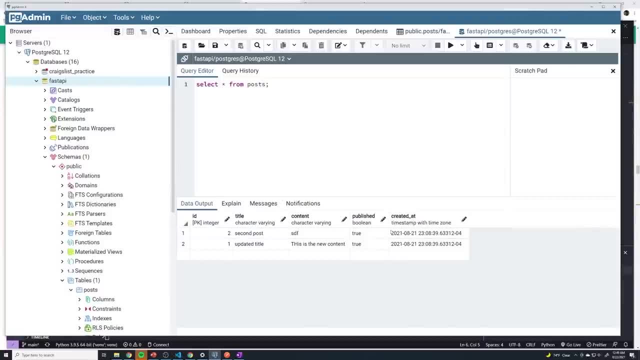 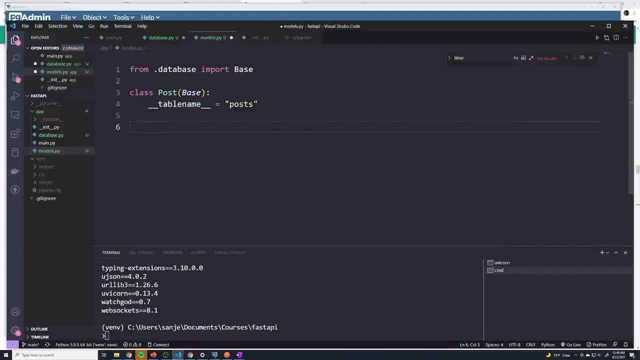 Right. So just like we went within PG admin and went column by column creating it, specifying all of their constraints and things like that, we're going to do this within, within our Python code. So we'll say: the first thing is we want an ID. So we'll say: ID equals. And then how do we actually? 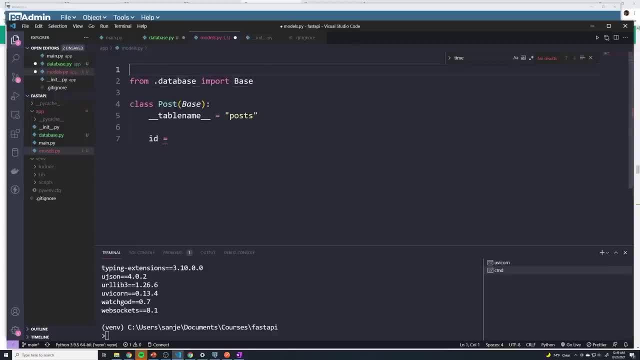 create a column. Well, we have to import something from SQL alchemy. So we'll say: from SQL alchemy, import column. So now I can create a column, And then there's a couple of different fields that we have to pass in. So the first thing is: 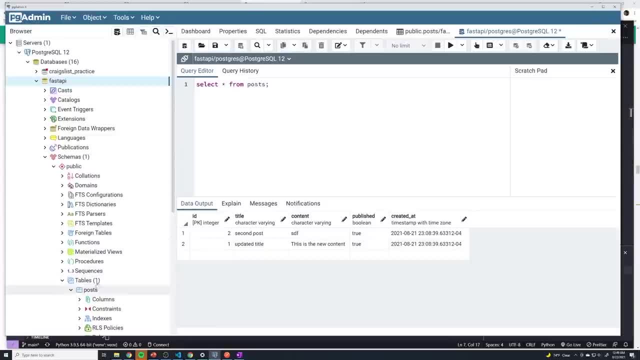 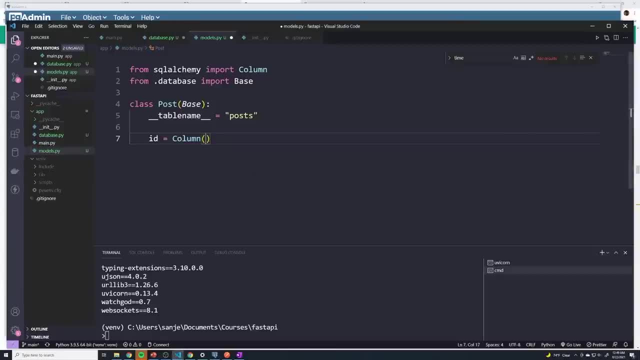 what type of column is it? And so if you go back to our post table and go to properties, right when we went into columns, the first thing they have to specify is what is the data type, And so we have access to most of the ones that we see in here. 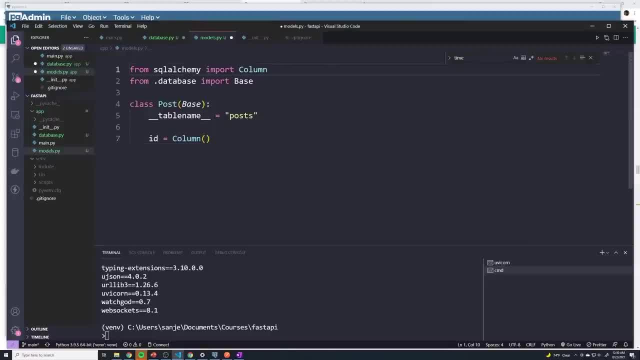 And. but we have to import it from SQL alchemy first. So the ID column is going to be an integer And so we have to actually import that. we'll do integer And now I can pass an integer. And that was a mistake. let me delete that. 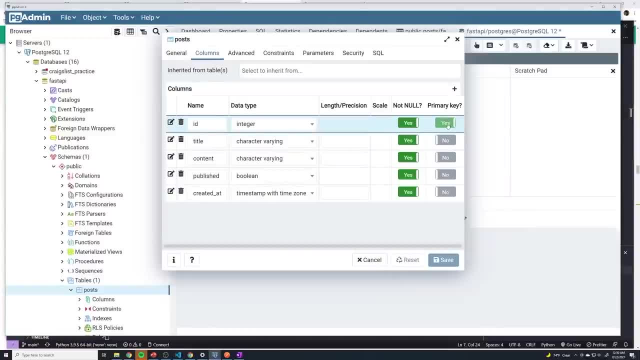 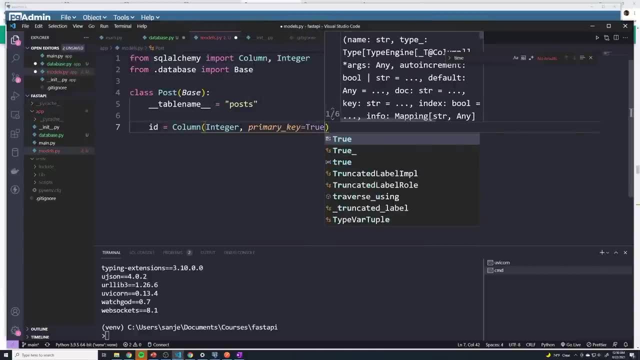 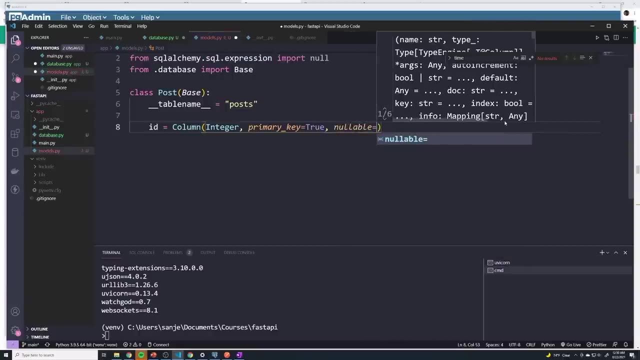 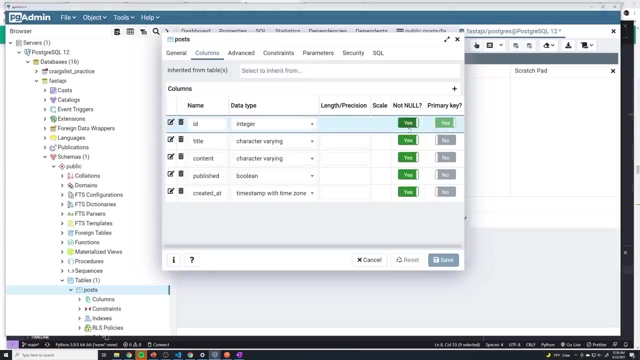 And then, if we take a look at our ID field, we did say that this was a primary key. So we'll say primary key equals true, And then, if you want to, you can also say nullable equals false, Right. so that's the equivalent of doing the not null. All right, then we can define the next. 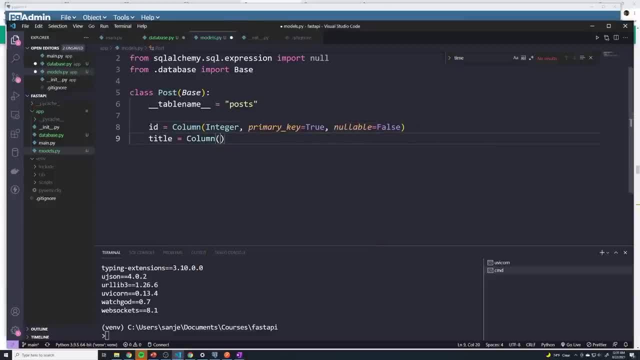 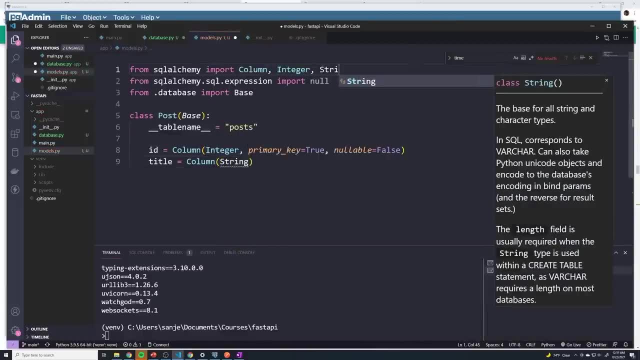 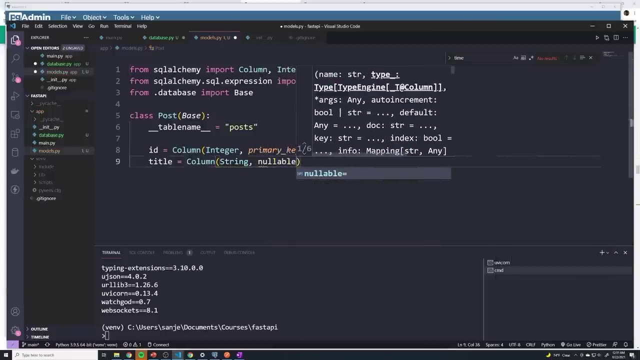 column was going to be title And then we call column. this is going to be a string now, But we have to import string from our SQL alchemy And once again this is going to be nullable, set to false. We can't leave that blank. The next column is going to be fairly symbol, similar. we've 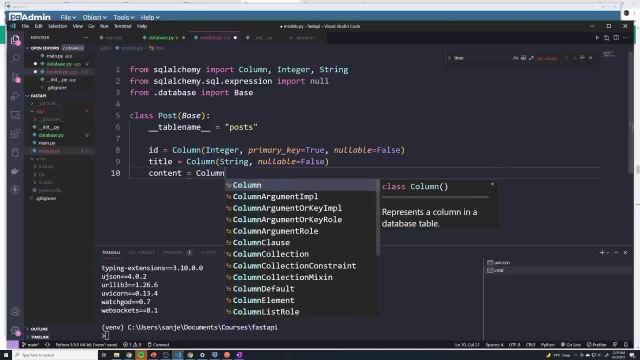 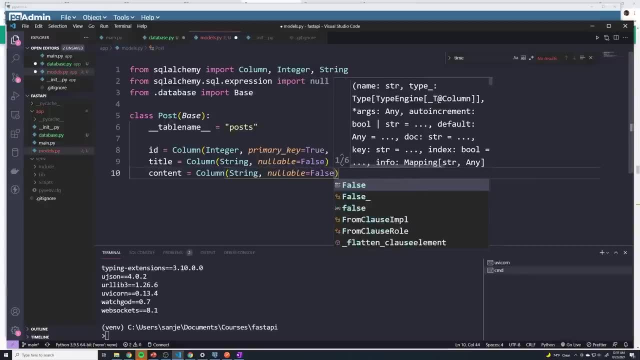 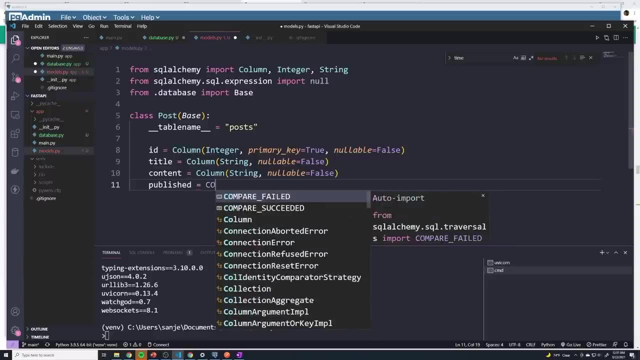 got content. This is going to be a string and nullable is going to be set to false. Then we got published This is going to be a Boolean, but we got to import that from the library And this one can be left as empty. 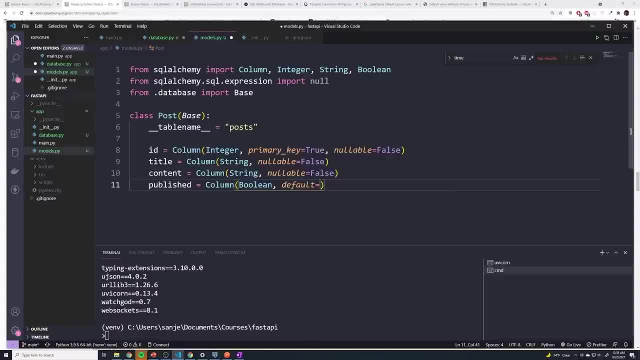 And, if you remember, we set a default value for our publish, So it's always going to be by default set to true if we don't pass in a value, And I believe that's how we do it. However, I'd have to double check just to make sure that's what it is. Now, the last column that we'll need: 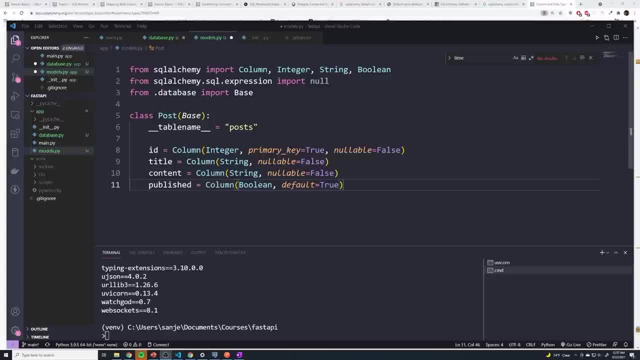 to add is the timestamp. But we're going to hold off on doing that for now And we're going to leave it as such And then later we're going to go back to our previous column And we're going to add the timestamp And then later we'll come back to adding that timestamp. in, All right? 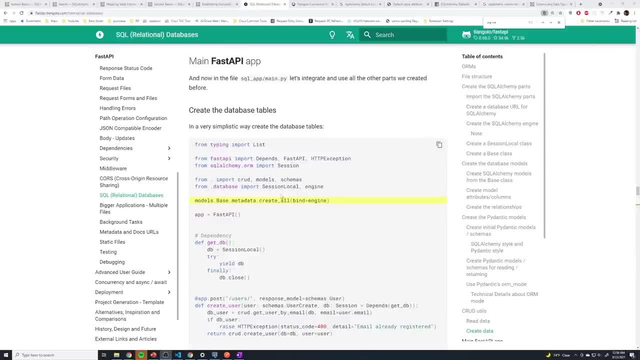 and so we're pretty much done with our model And what we want to do is in our main file. we want to copy this command right here. So this create engine, so this is going to create all of our models, So we'll go to our code, we'll go to my main file And somewhere up top, 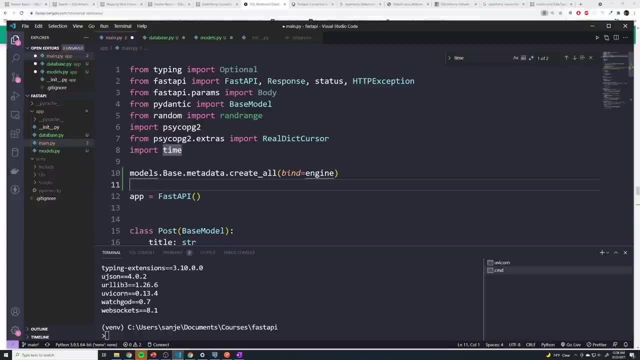 I'm going to create that right there. However, we have to import the right commands, And so the first thing that we want to import is our model. So we'll do from star import models, And then from our database file, we'll say from: 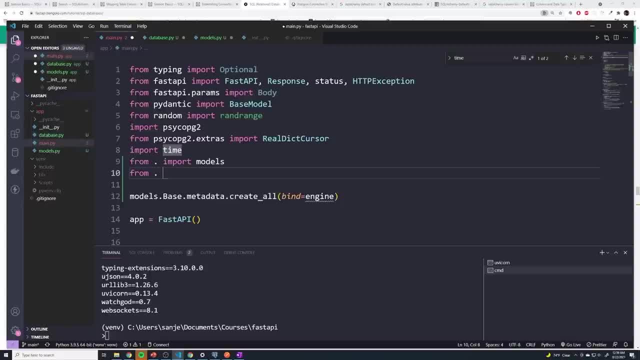 dot, which is current directory. So we're going to grab a file from our current directory. we're going to import- Sorry, from our database file, we're going to import engine, And so at that point that is good to go. 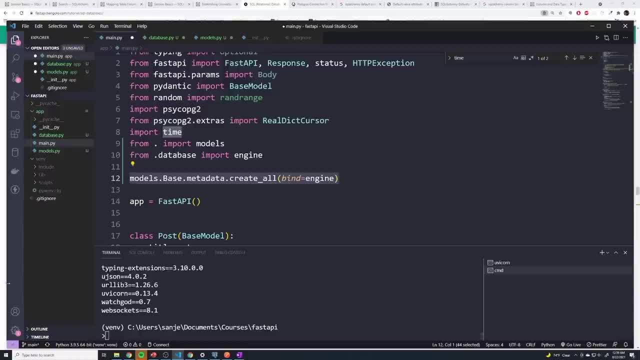 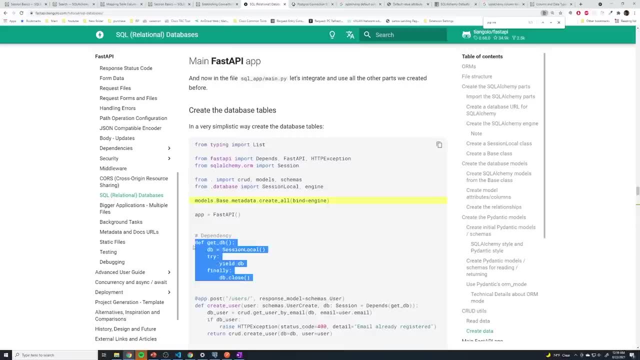 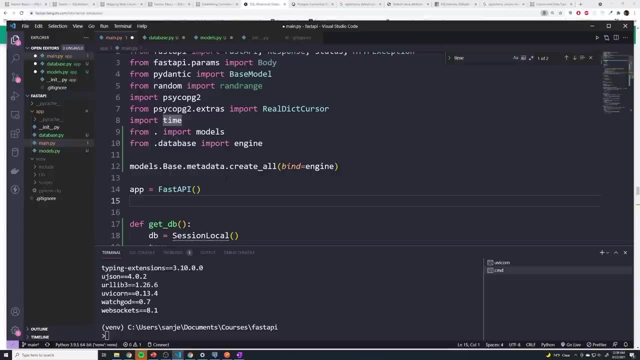 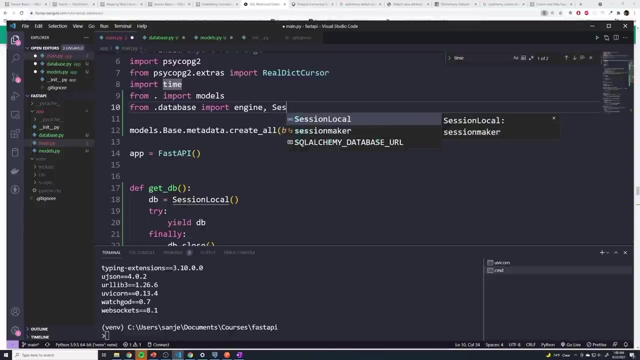 And then, finally, if we go back to our documentation, the last thing that we have to do is we have to create this dependency. So just go ahead and copy this for now And just paste it in here, And we want to import session local as well, And we should no longer get any errors here. 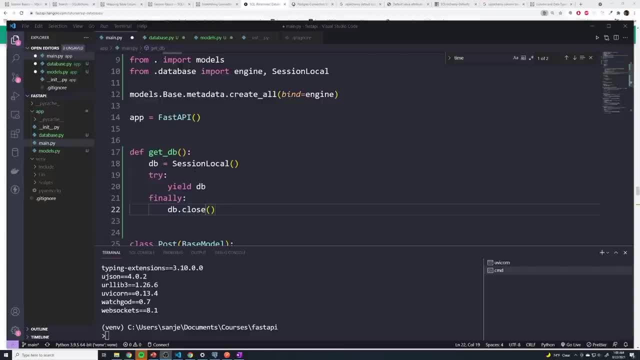 And so what this ultimately is going to do is the session object is kind of what's responsible for talking with the databases, And so we created this function where we actually get a connection to our database or get a session to our database, And so every time we get a request, we're going to. 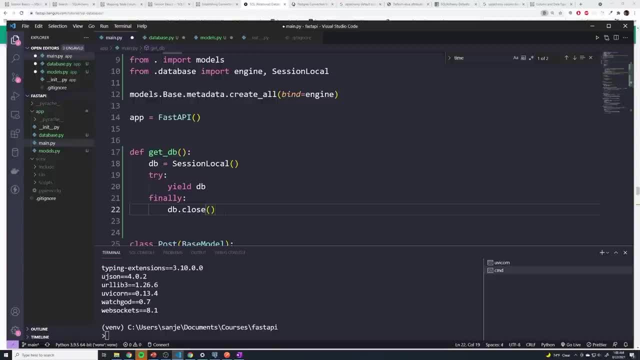 get a session we're going to, you know, be able to send SQL statements to it, And then, after that request is done, we'll then close it out. And so it's as much more efficient doing it like this, by having one little function And we can just keep calling this function function every time we get. 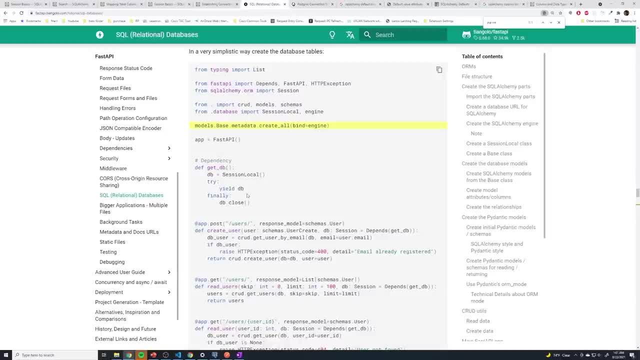 a request to any of our API endpoints. So that's what we're going to do, And then we're going to create our session. And so, now that we've got our dependency, to actually get that session for all of our path operations where we want to perform some sort of operation on the database. 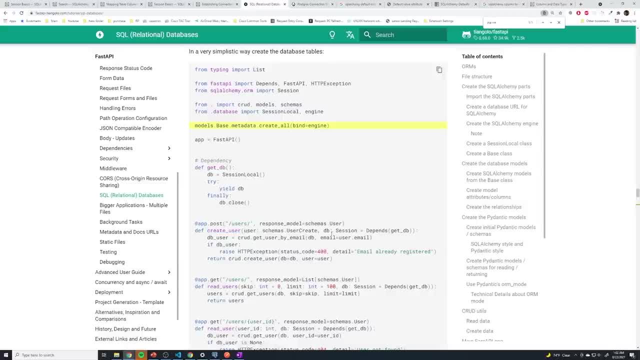 what we're going to do is with with inside the path operation function. we're going to pass in another parameter and it's going to be session equals depends, And then we're going to call this get DB function. So what that's ultimately going to do is this line right here, don't worry too. 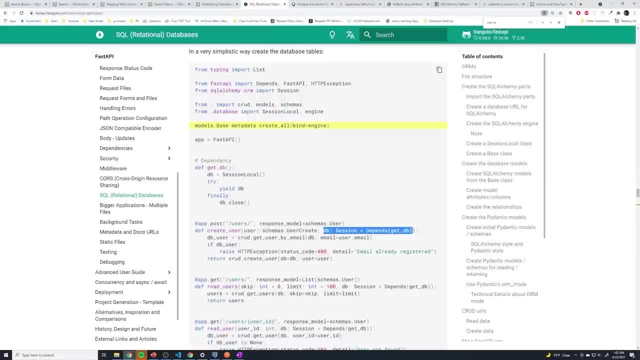 much about it. But, like I said, it's going to create that session to our database that we can perform some operations and then close it once that request is done, And then we're going to repeat that process for every single one of our path operation. So anytime you send a request to 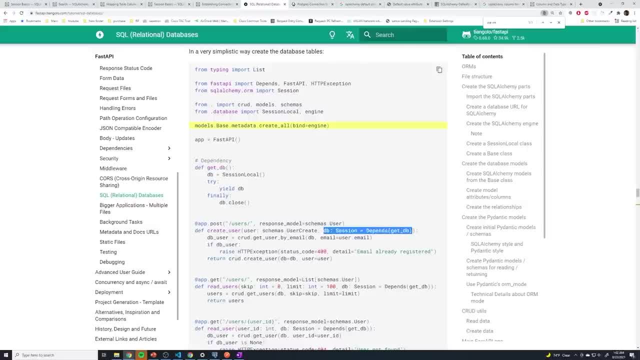 any API endpoint. you're going to have this being passed into the path operation function so that we can create that connection and then close it out. And, like I said, a lot of this is just copy and paste. So once you write this down, even if you don't really understand it, you don't really have 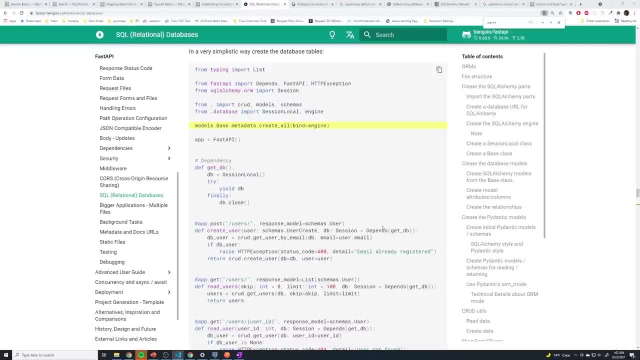 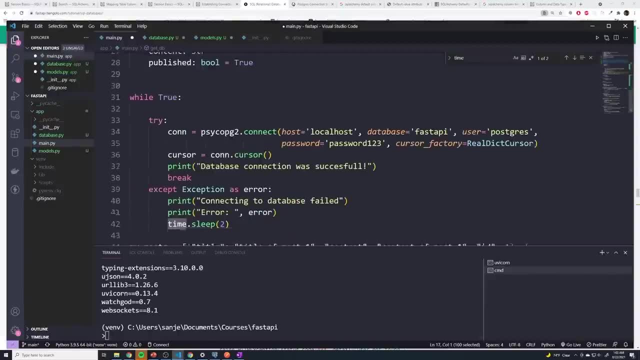 to touch it ever again after that. Alright, so let's copy this, And what we're going to do is I'm going to create another route Or another path operation, just for testing purposes, because I don't want to mess up any of our other. 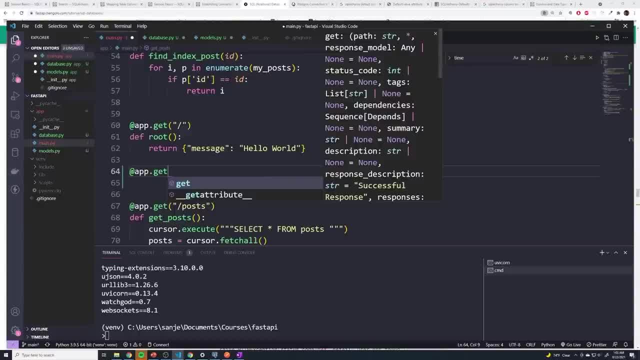 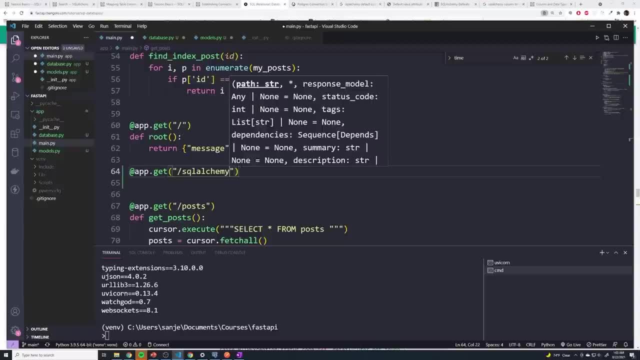 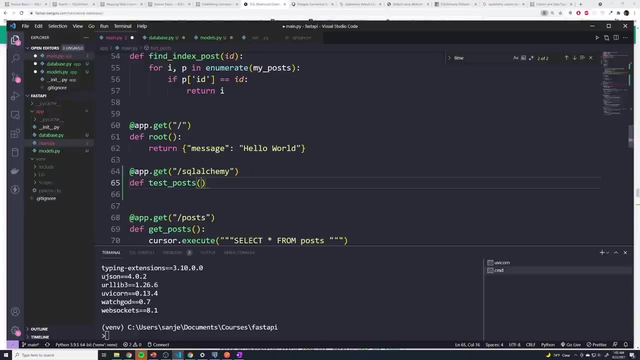 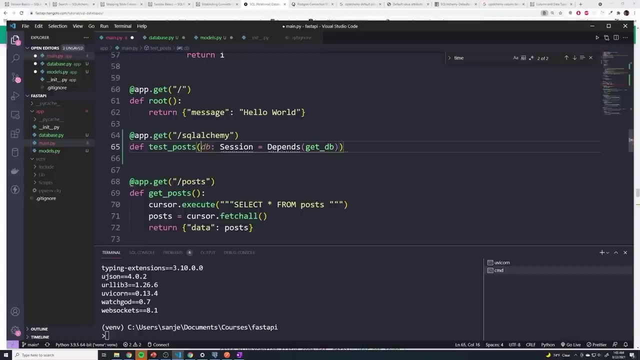 code. And so I'll just say at app dot, get And this is going to be at slash SQL alchemy. So this is just a test to see if it works, And I'll say def test posts And then we want to pass in that, that code. 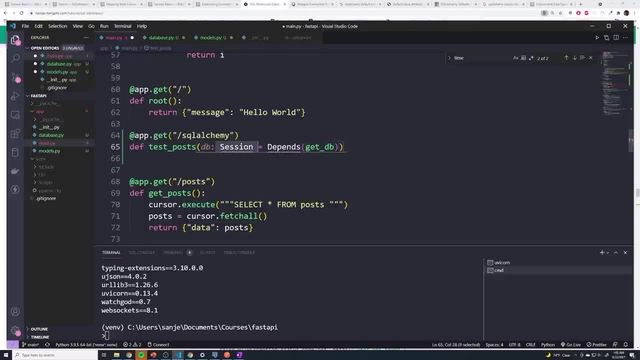 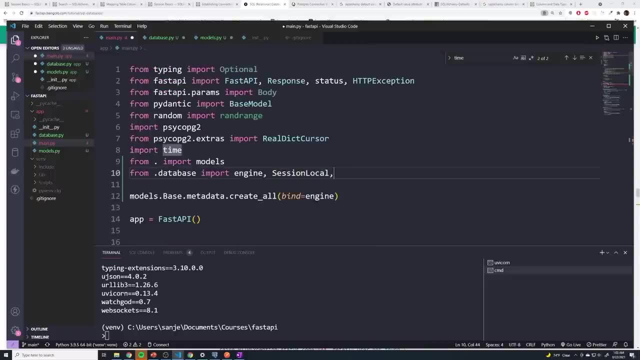 that we just copied right here. However, we don't have a session, or depends in this case, So we're going to have to import those. So from our database file, our session is going to be from there. Actually, sorry that's. 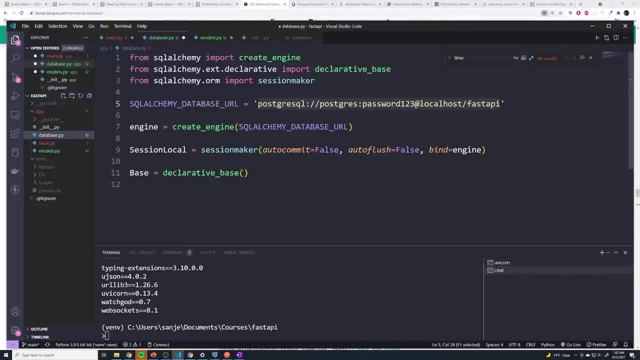 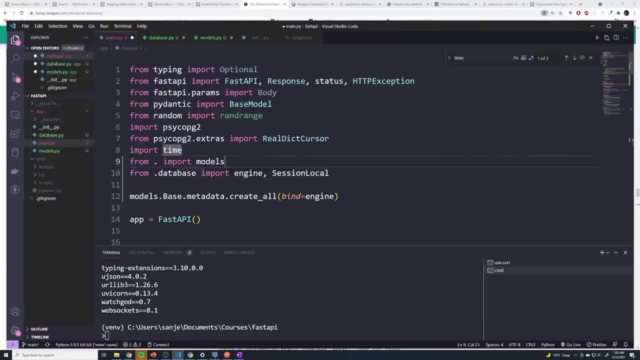 not actually coming from there, Is it? Do we have a session in here? We actually do not have session here, So instead, this is not going to come from there, Actually, instead we're going to import that from SQL alchemy. 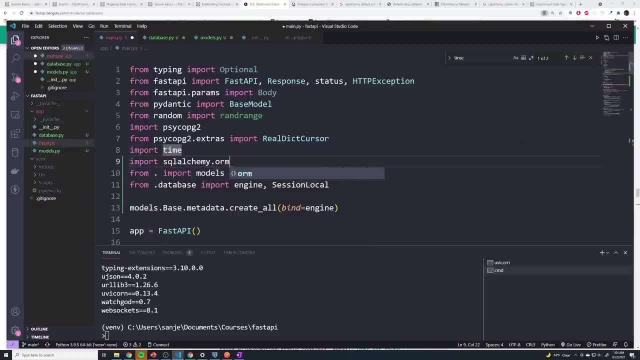 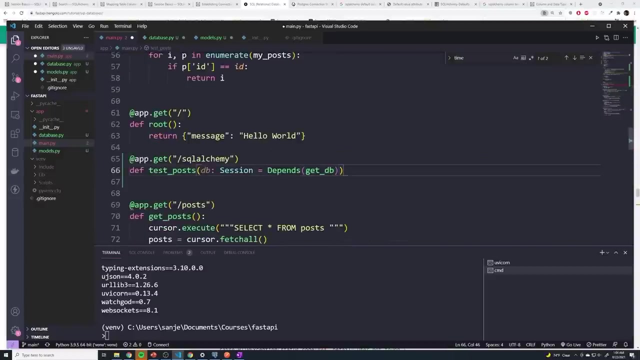 import session And I realized this should be a from. And then we also have to import the depends method from our fast API library. And so now, if we go down to our route, we should get no more errors and it looks good, And then here we're just going to return. 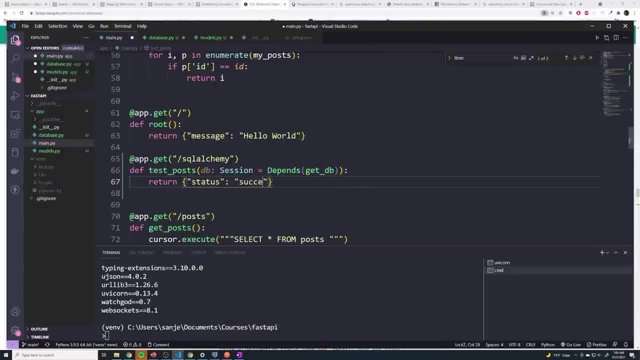 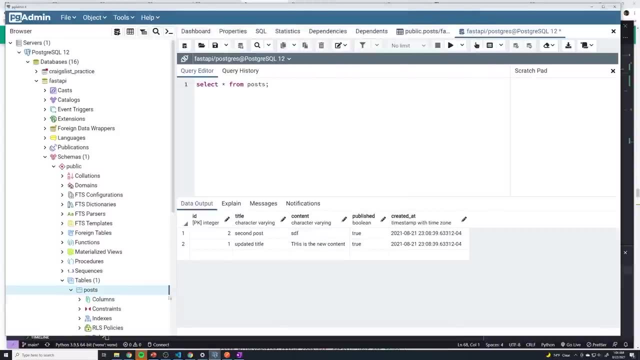 status: Success for now And then. finally, the last thing that we're going to do is we're going to delete our post table. I'm going to do a delete, Drop it, Yes, And we have no more tables. Now I can close this out. 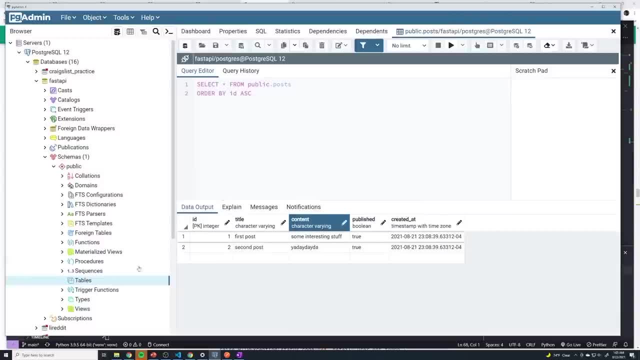 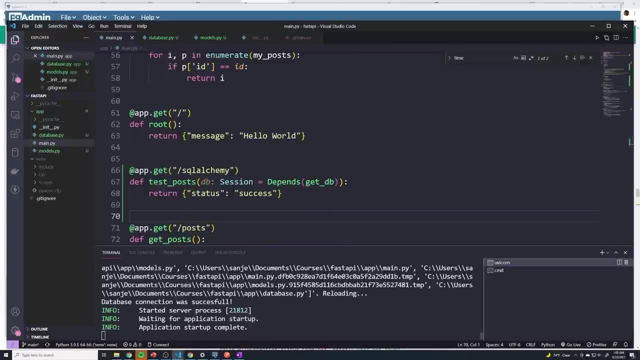 I didn't mean to save that close that. don't save it, I'm sorry. no errors. Right now we've got nothing, So let's save everything And pray to God that there's no errors. and so it doesn't look like there's any errors. 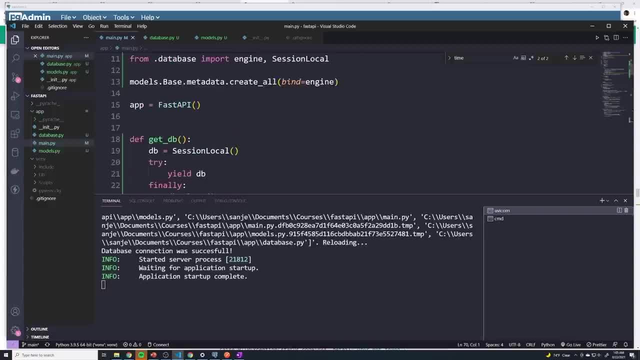 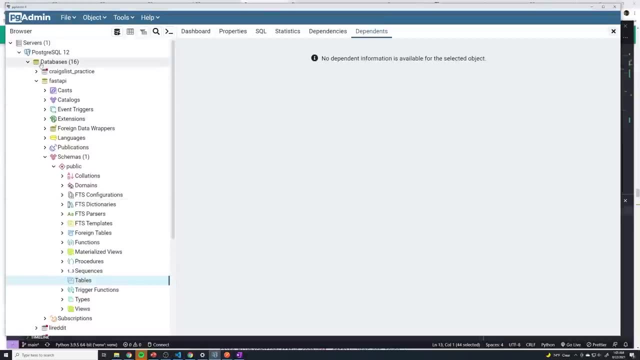 And just by saving that code and restarting our application, what should have happened is, once our code ran and we run this, I believe this should actually create the tables within Postgres. So let's refresh this real quick. I'm just going right here. 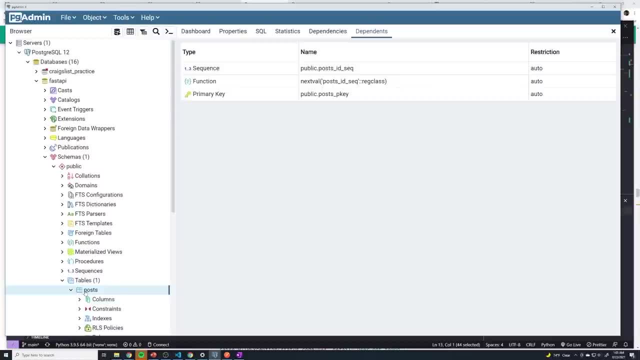 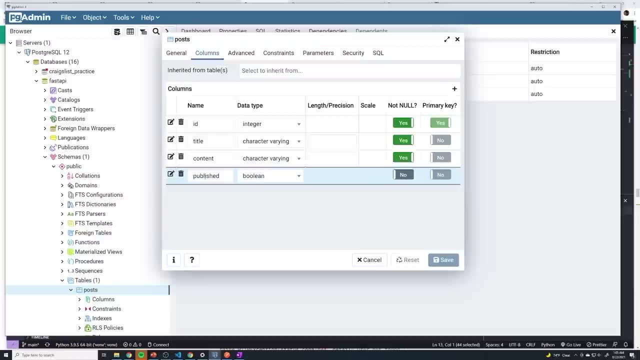 hit refresh. look at that, guys. we now have our post table, even though we deleted it. So if we take a look at our post table and go under properties columns, you could see it's got the three columns that we define, all four columns that we defined And that all comes from our modelspy. 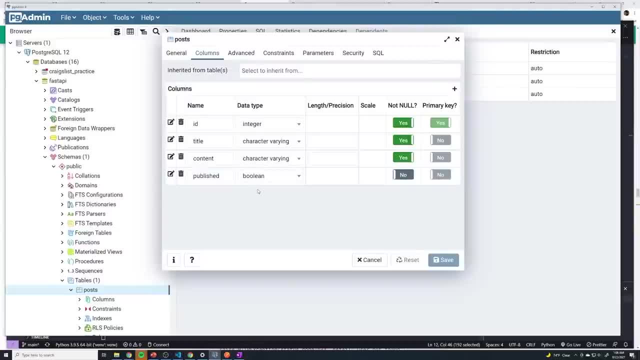 And so we've got the four columns that we defined here, And so if, whenever we start our application, SQL alchemy will check to see if there's a table called posts. If it's there, it's not going to do anything. If it's not there, it's going to go ahead and create it for us based off of what we 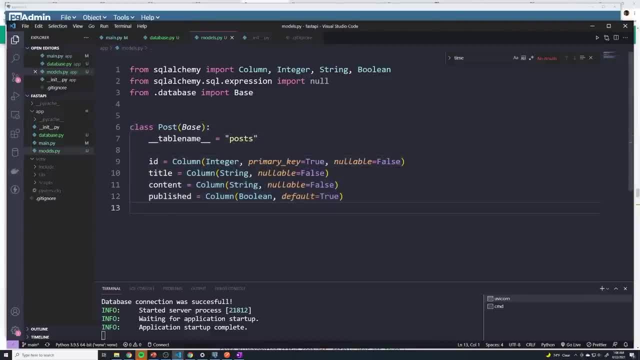 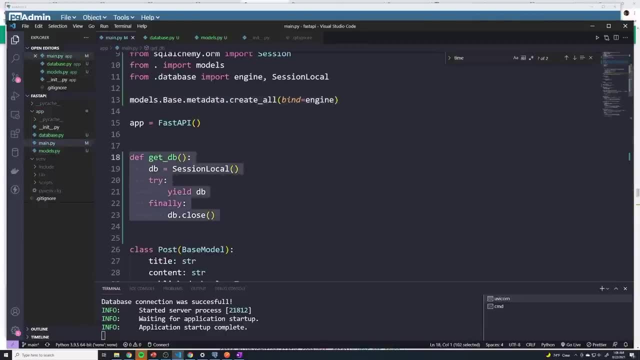 defined in the model. Now there's one last thing that I want to do, just to kind of clean things up in our mainpy file. I don't like having this get DB function within here. I want to keep all of my database code, all of my database initialization code, within my databasepy file. So what I'm 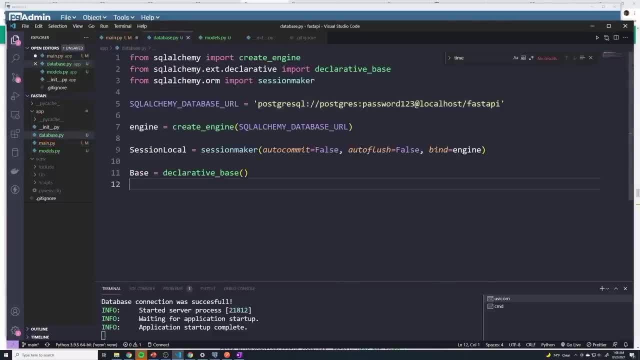 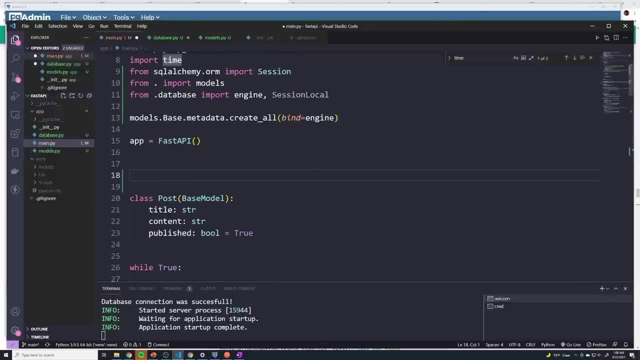 going to do is I'm going to actually cut this out, paste it into my databasepy file And then we're going to import this into my main file so that I don't have to have that in my main file, cluttering it up, because our main file is already fairly large. So for my database file, 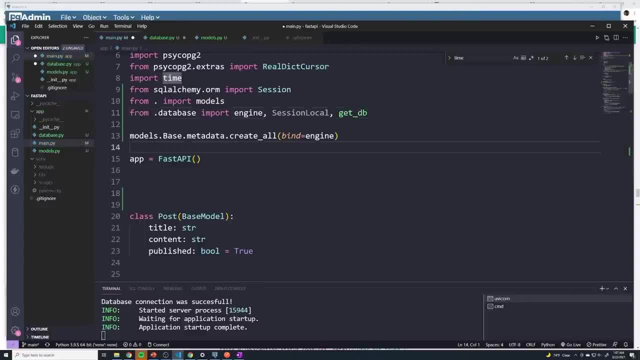 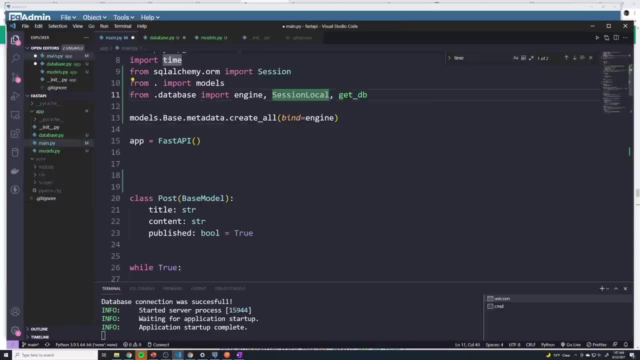 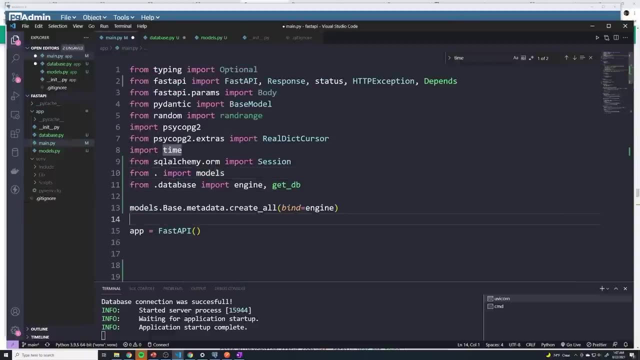 I can import, get underscore DB And now we no longer need session local because it's showing us it's grayed out, So we can remove that And at that point everything should be fine. It's still be working. So, just as just to double check, I'm going to delete this once again. 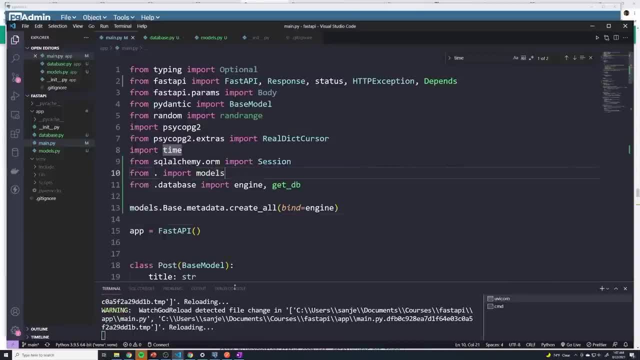 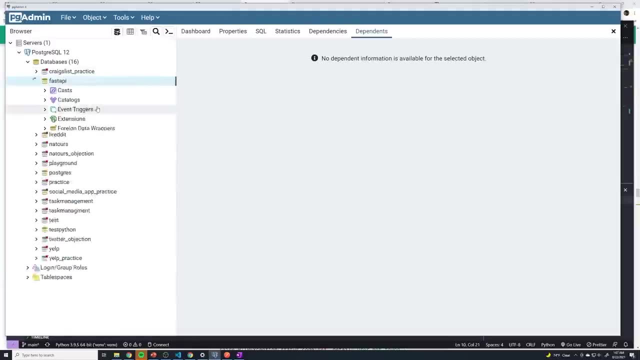 And then I'm going to save this, which is going to trigger a reload of our application, And then, once our application reloads, if I refresh my database, it should have created another day another post table, and it looks like it did, And let's just double check that all of 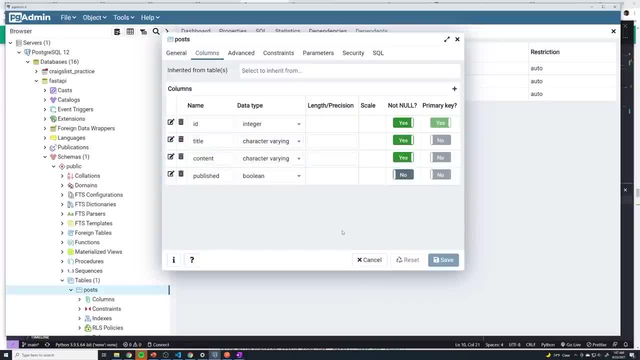 the columns are there And it looks like they are, So everything looks good. In the next video. the one thing that we do need to change is that we have to add the created at column, So we'll tackle that in the next video. In the last video, we were able to get SQL Alchemy to generate. 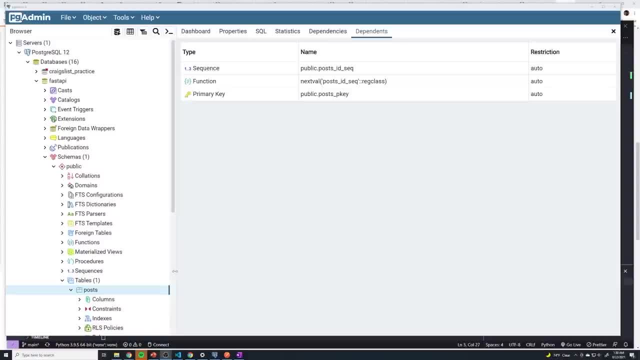 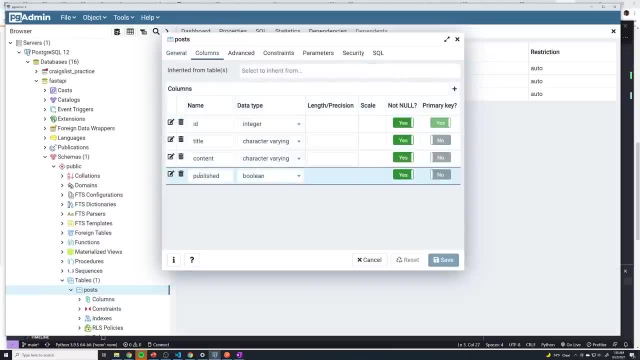 our own post table. However, if we actually poke around with it, we'll see that there's a couple of issues. So if I go to right click on it and select properties and I go to columns, all right, we can see that all of these fields are set to not null And the primary key is set. 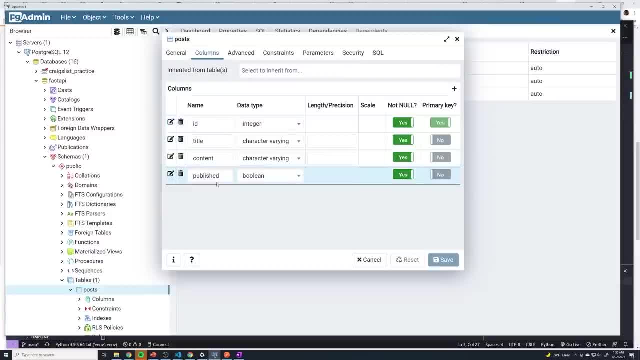 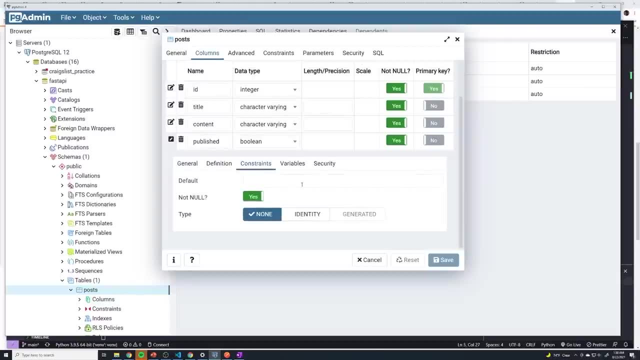 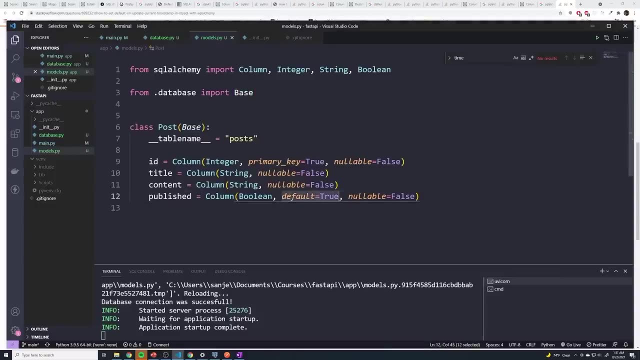 to the ID field, So everything looks good so far. However, when I go to the public published column and I go to constraints, I can see that the default isn't set, And so if we go back to our code, I actually made one little mistake, right? this default is not going to. 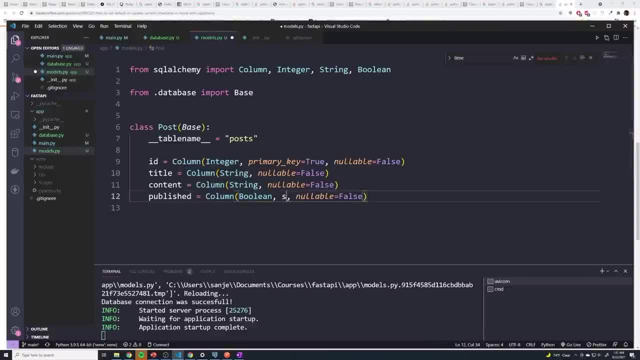 give us what we need. Instead, what we need to do is we need to set this to server default, because it's ultimately the, the Postgres server or the database server that's going to actually send the default. So I'm going to put it in quotations As a string. we can just set this. 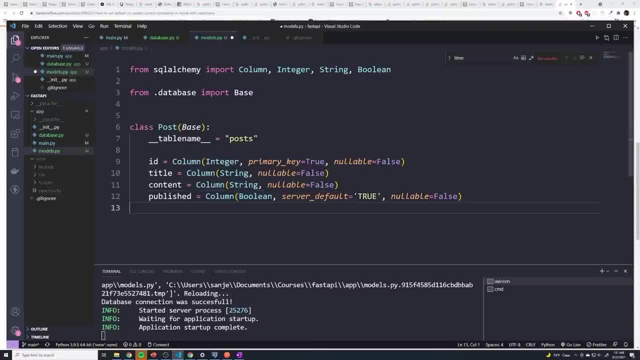 to be true And then, if you haven't added this, go ahead and add nullable to false. I'm going to make all of my columns not allowed to be empty. That's because the server is going to add the default to true for this. So let's try this out Now. if I hit save right now and I go to my Postgres database, 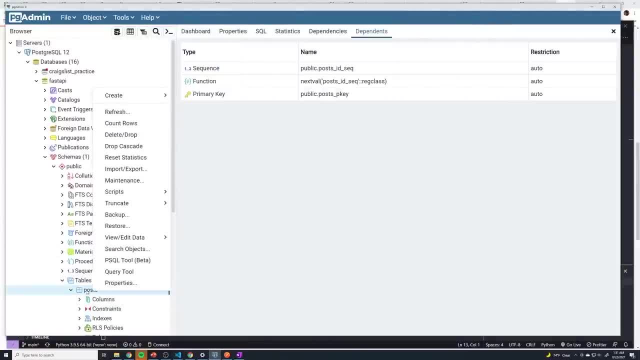 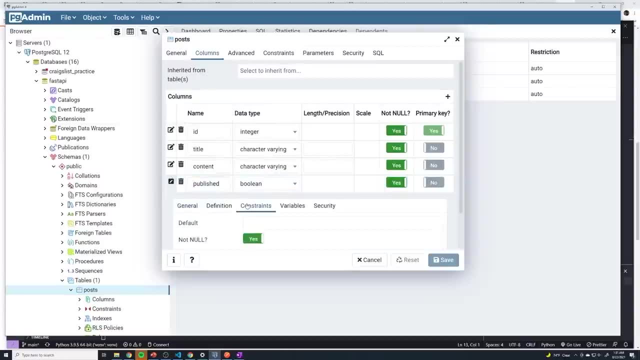 and then we can just right click on this, hit refresh, And then we do properties again and I go to column And then we go to- sorry, go to the publish column. we'll see that there's no constraints, And so this is kind of a limitation of SQL alchemy. 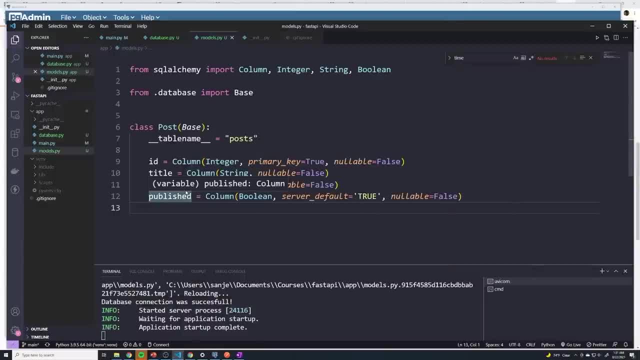 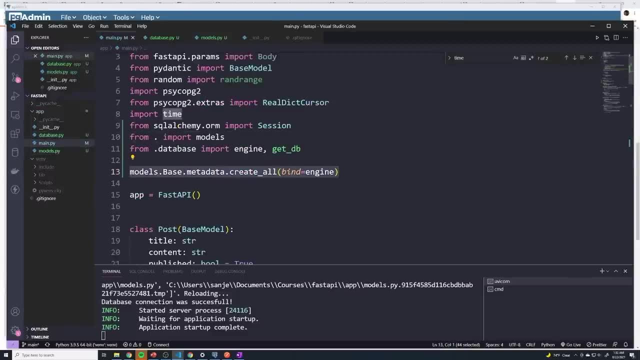 because SQL alchemy will generate your tables, But it does it in a very simple manner. What it actually does is if I go to my mainpy file and then it runs this code: I believe this is the code that actually creates the tables. What it does is: it'll go through all of our models and it'll look. 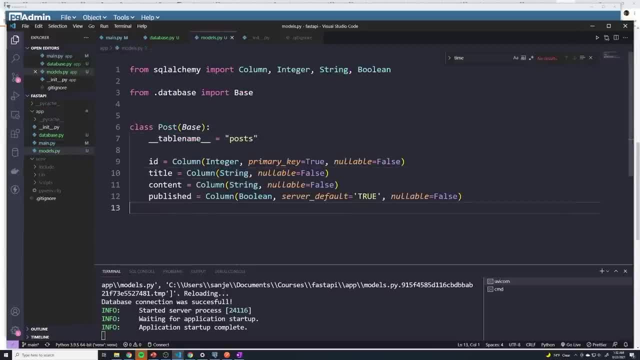 for a table named called post. If it doesn't exist, it will then create one based off of these rules. However, if the table already exists, even though we've changed the different attributes, columns and things like that, if it looks for the, if it finds a table with that name already in 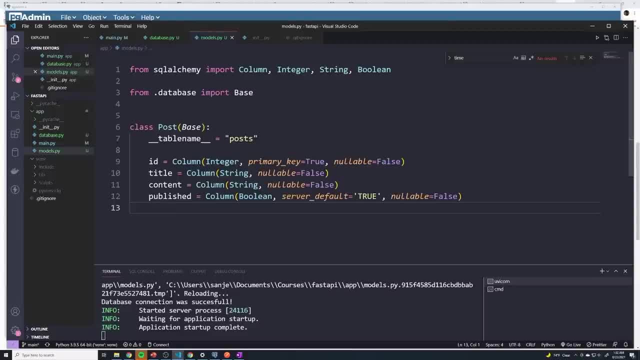 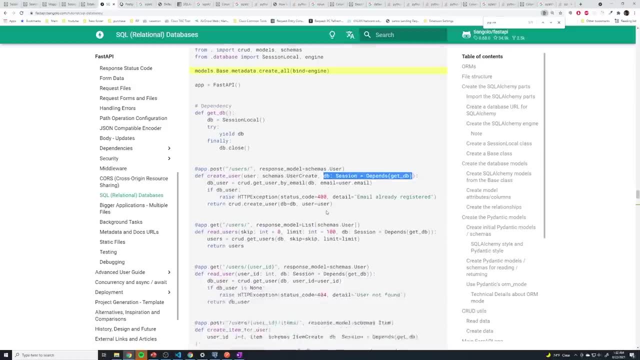 there. it's not going to touch it, So it's not going to help us modify tables and things like that. In fact, if you actually take a look at the documentation, I've got so many tabs open. let's see if I can find it right here And search for alembic And so normally, 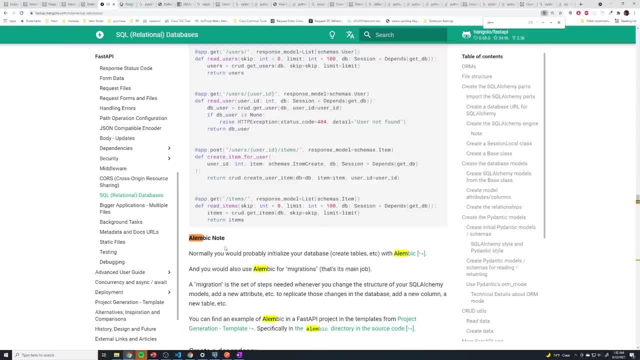 when it comes to creating your tables. when it comes to handling migrations, which is a term that's used for changing the columns and the schema of your tables, then you want to use a software called alembic SQL. alchemy isn't really meant for handling database migrations or making 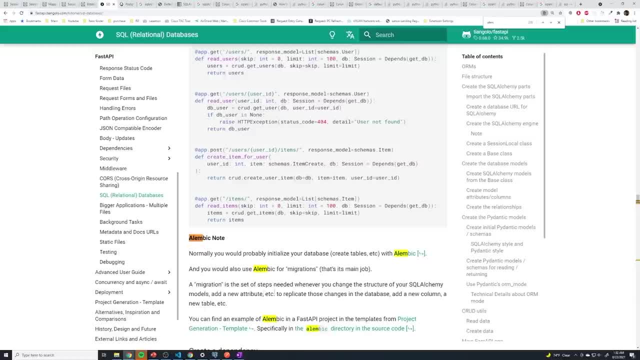 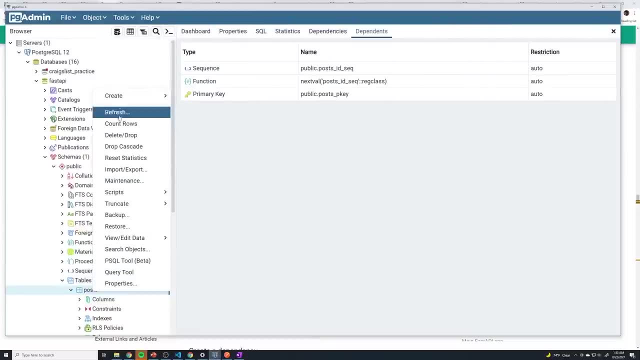 changes to it. So that's why we don't see it automatically make those changes. So for now, what we're going to do to get around this limitation is: I'm just going to cancel out of this and we're just going to delete the table. So we'll drop the table And then we'll go back. 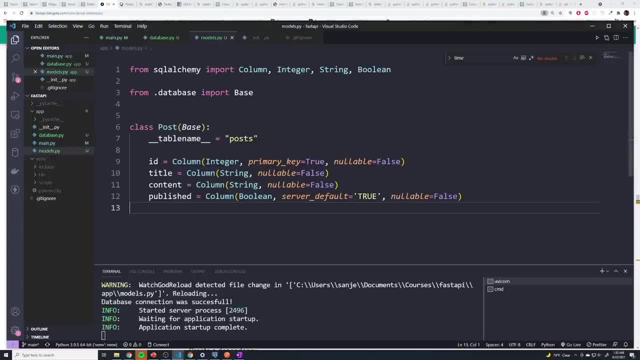 to our code And I'm just going to hit save And so, now that it runs again, it's going to look for a table called posts, Since we deleted it. it's not going to see it. it's going to then go ahead. 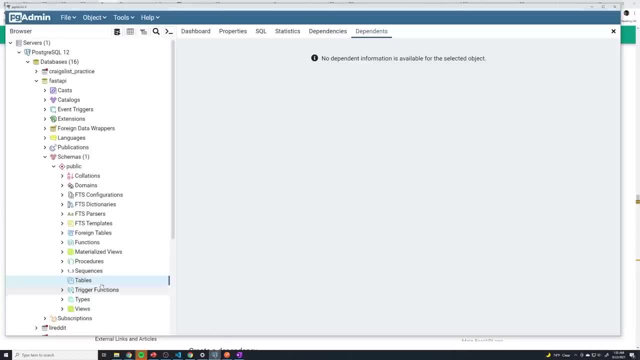 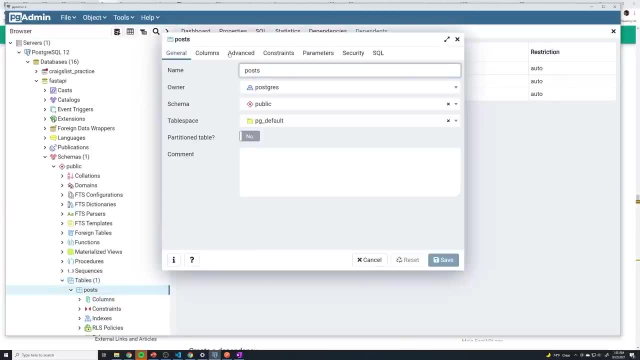 and create our table. And now, if I just right click on tables, hit refresh, we should see that we have a post table And if I go to properties, we can then go to columns published And if we go to constraints, 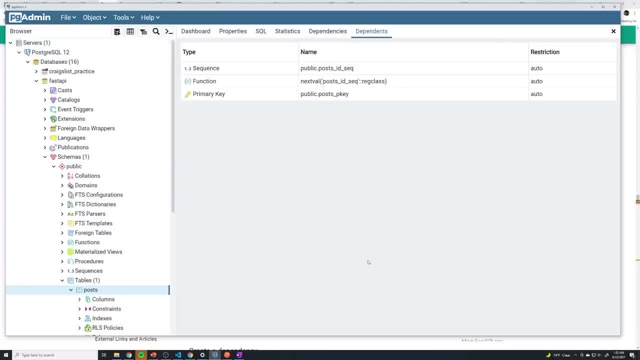 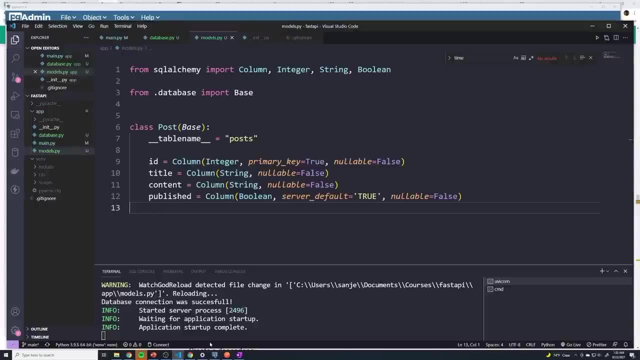 we can see the default set to true, So it looks like that. fix that issue Now. the second thing I want to do is I want to add our timestamp column, because that's very important. we need to know when a post was created, So let's create a field called created- created- underscore at. 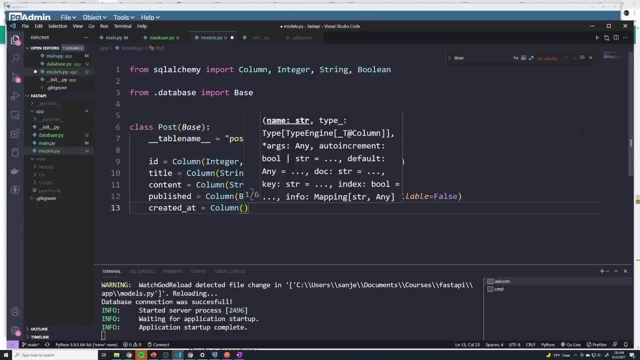 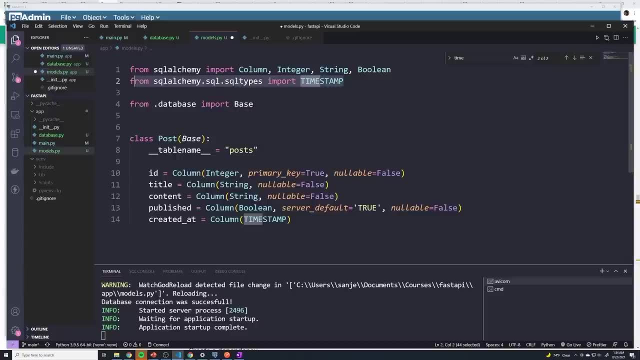 column. Now, what's the column type going to be? Well, we're going to use a column type of timestamp, So type in timestamp. we can let VS code automatically import it. But all it's going to do is it's going to import it from SQL, SQL, alchemy dot, SQL, dot, SQL types, And then within. 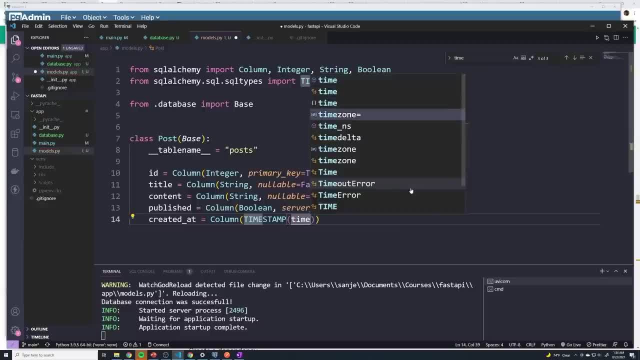 here we have to pass in a property of timezone. equals true, So this is going to also add in the timezone And that's going to be a capital T, And the next thing we want to do is provide a. it's going to be. 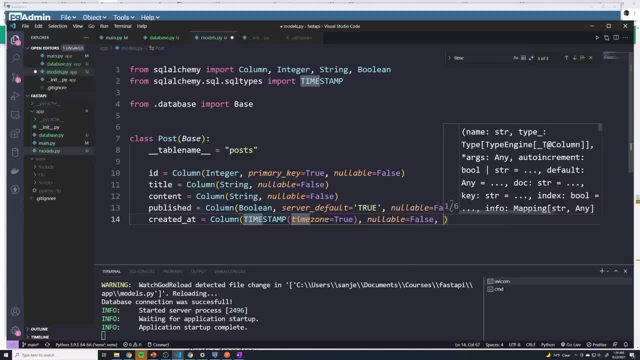 nullable, set to false, So it can't be left empty. but we're going to give it a default value if the user doesn't provide it, which they never will, And so we'll do server default. But we have to do something a little bit different here. I have to import a function or a method called text from. 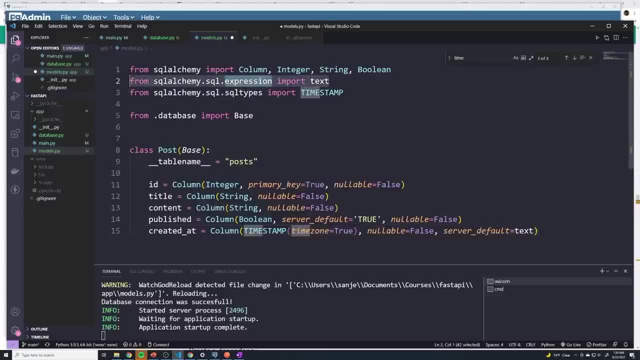 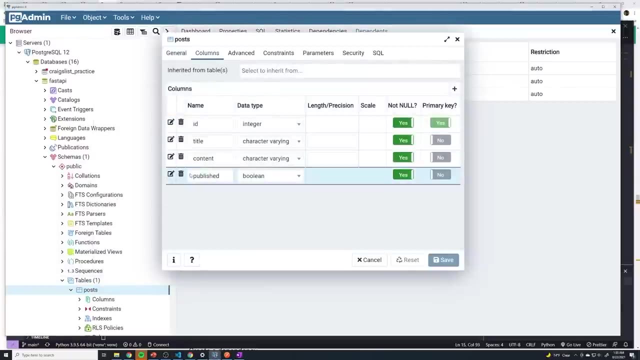 SQL alchemy. So from this right here, SQL alchemy, dot, SQL dot express. I'm going to do text And then here we're going to do now right, just like we typed in within our Postgres database. You know, if we wanted to manually do this, we would just go under the column let's. 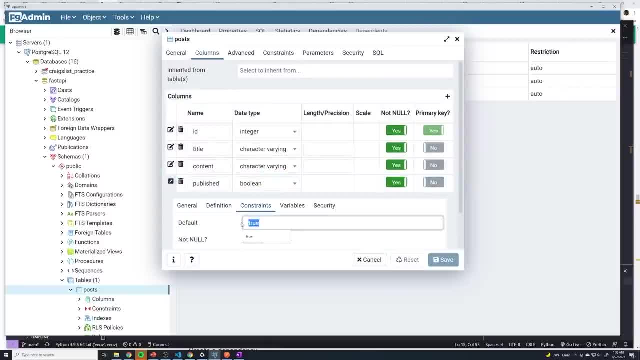 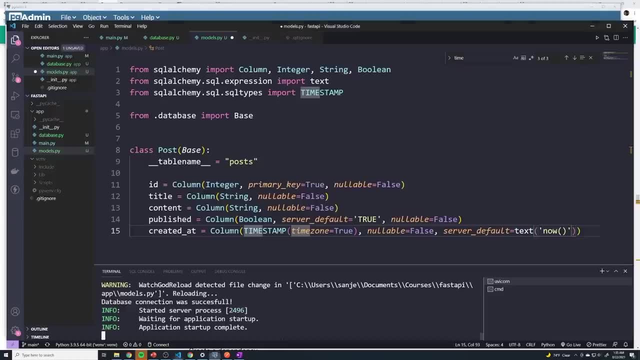 say, we had to create a column. we can just go in there, go into constraints and then type in now like that, And that's going to generate a timestamp. So we're doing the same thing, But we're just doing it through Python code now. So once again, we'll save this. I'm going to drop this. 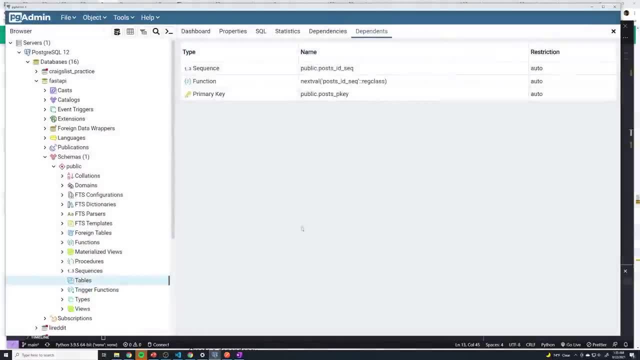 table so that we recreate it And then we'll save it one more time. this is going to trigger a reload and then a refresh of the table. we should now see it. So let's go into properties. Let's take a look at our columns. we've 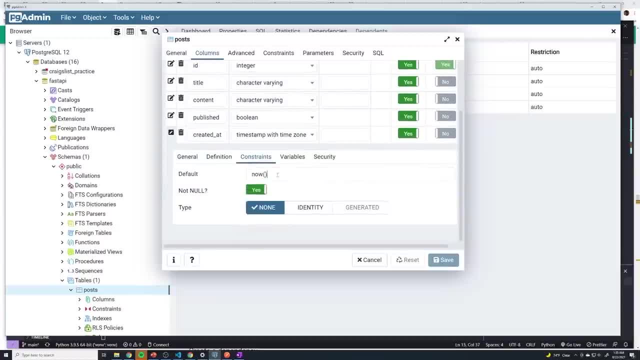 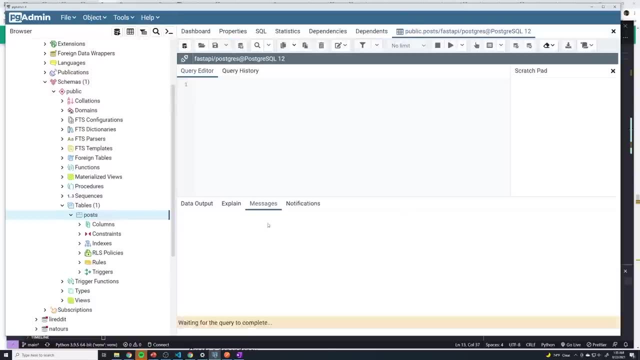 got the created at column And then, if I go under constraints, we can see the default is now set to the current time. So we've got that working. Let's just quickly test this out. So I'm going to go into view, edit all rows And I'm just going to create a post. 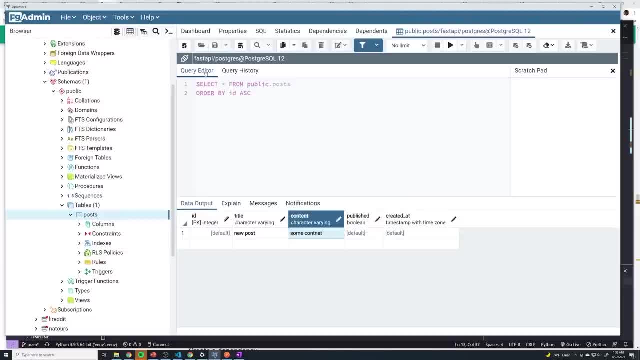 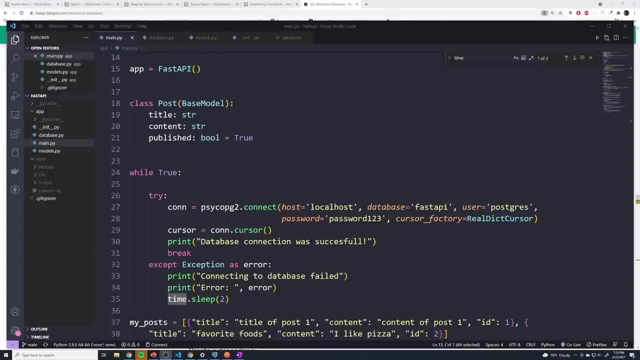 We'll save this and let's make sure all of the default values gets. it looks like that's good And it looks like the time is set just right as well. So now that we have verified that SQL alchemy has created the proper tables within Postgres, it's time to go ahead and create our first query, And 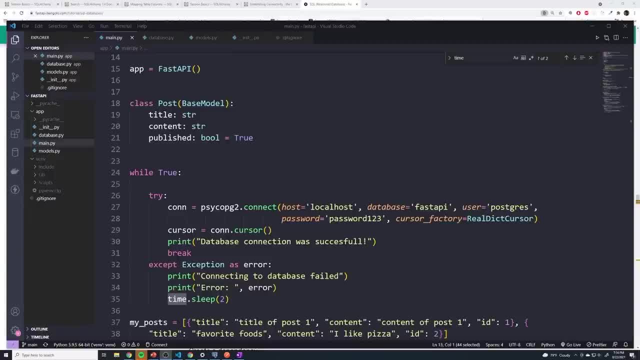 like I mentioned in a previous lesson, with SQL, alchemy or really any ORM, the way we do queries is going to a little bit, is going to be a little bit different. we're no longer going to rely on regular SQL. Instead, we're going to rely on regular SQL And we're going to rely on regular SQL. So 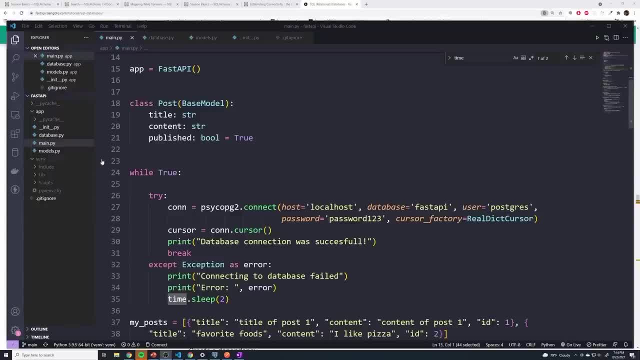 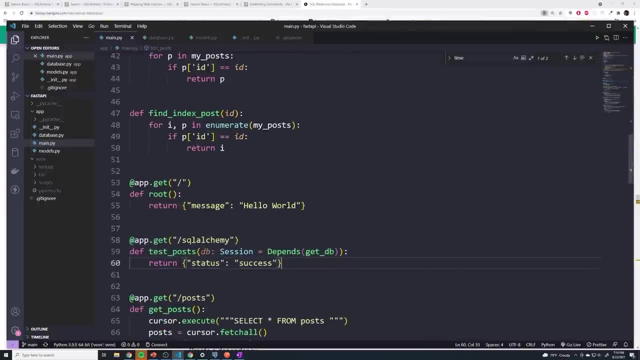 we're going to use basic Python methods And so go to your main folder- sorry, your main file, right, And we? we saw this test route that we defined. So what we're going to do is we're going to run our first query within this test route And then afterwards we can go ahead and 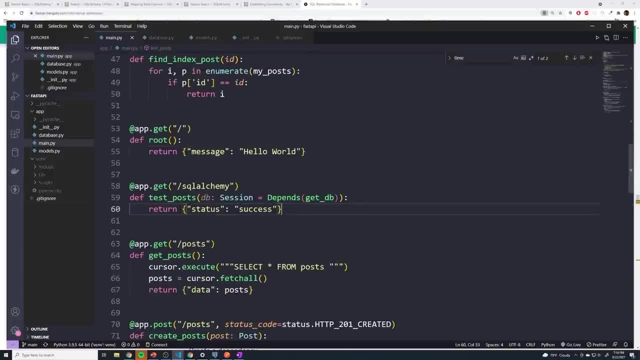 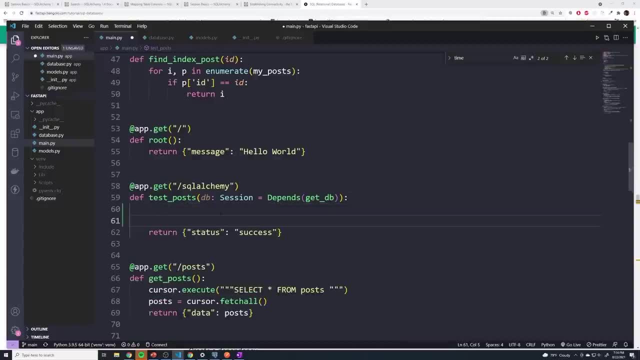 delete it, And then we can update all of our pre existing path operations. And so, like I mentioned before, anytime you want to perform any kind of database operation with SQL alchemy within fast API, we want to make sure that we pass it as a test And then we're going to run our first query. 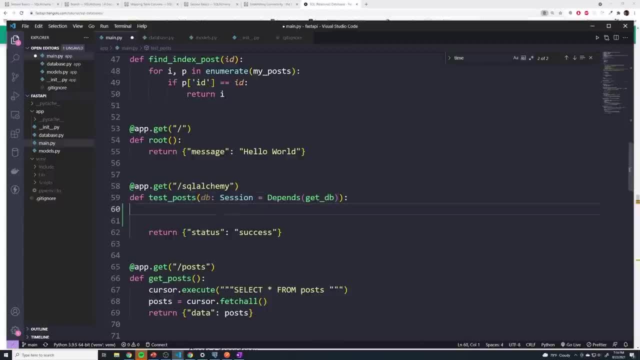 as a parameter into our path operation function. So you just call DB, So we're saving it inside a variable called DB And then we're just calling the session object And then we're calling the get DB function within depends. So this makes it a dependency, And so if you already forgot what that 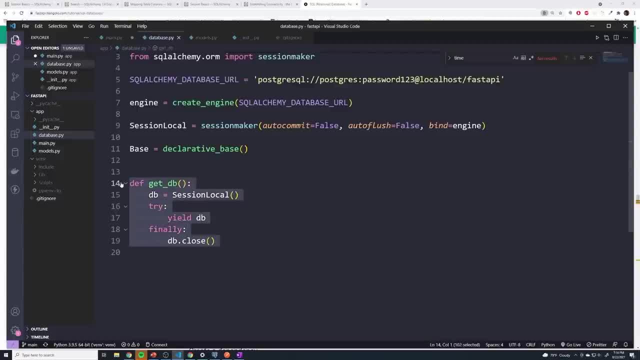 is just go to your database. you can see that it's this function right here. So this is going to actually create a session towards our database for every request to that specific API endpoint and then it's going to close it out once we're done. 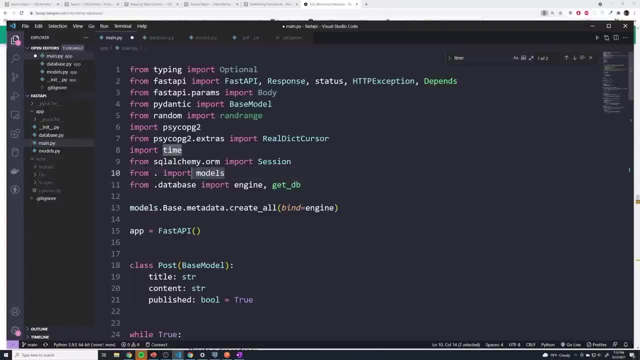 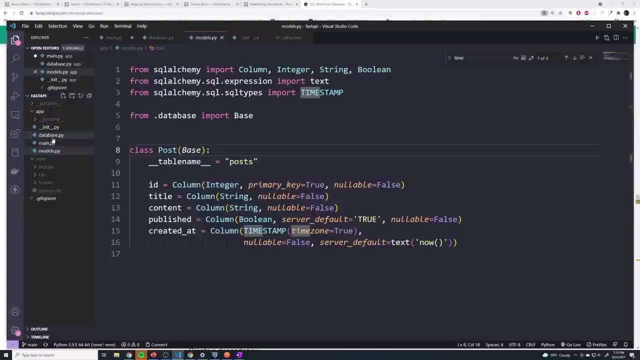 Right, And then within main, there's one thing that we have to import and that is models. So you just do from dot import models. that's going to import this specific model so that we can actually make queries to it. Right, And to make a query, right, we're going to access that database. object: 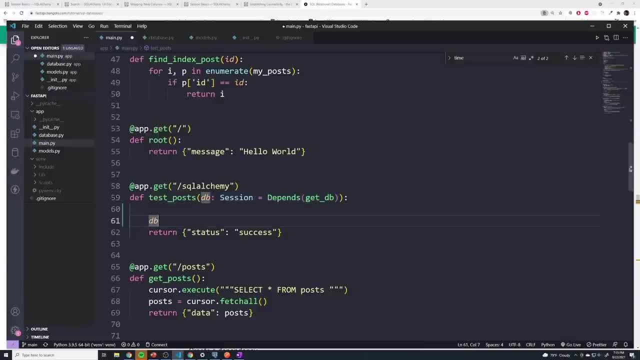 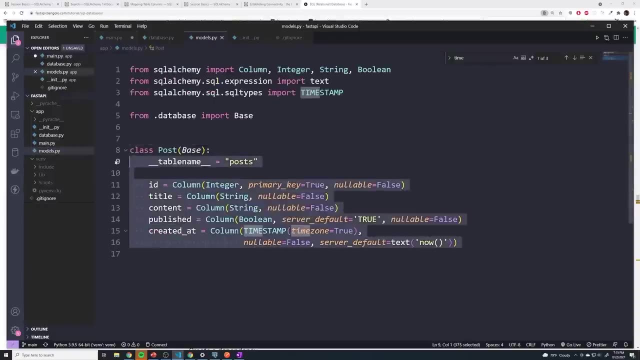 which is getting passed into our function, And then here we want to tap into the query method And then we have to pass in the specific model for the table we want to query. we only have one model in this case, which is our post model. 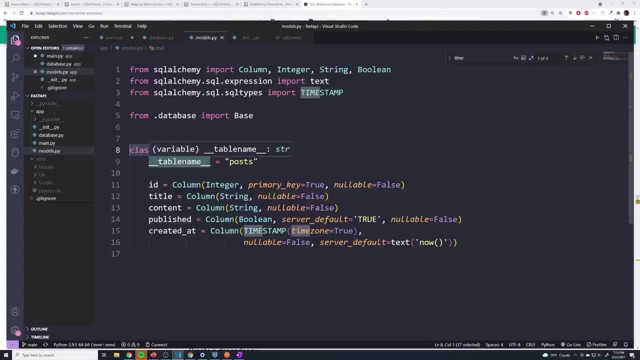 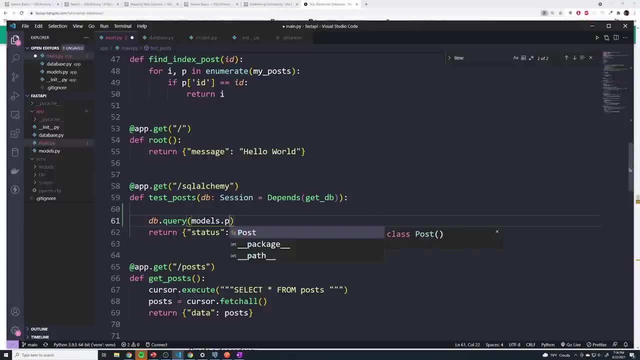 So that when we use this specific model, it's going to allow us to make a query to our post table, And here, so we'll call models dot post, So that's going to allow us to access that model. And then, from here, what we can do is we have a couple of different methods that we run can run, But since 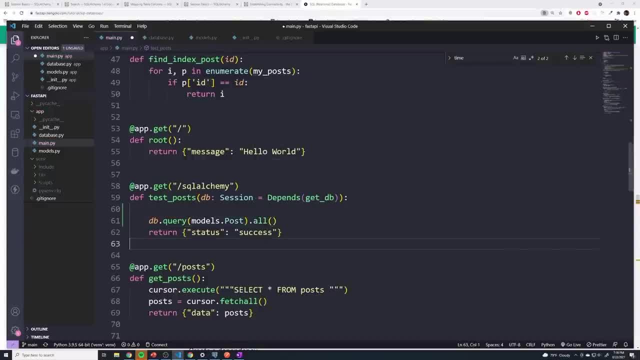 we want to query all of our posts. we just do all those is going to grab every single entry within the post table And then here we could just save this as a variable called posts And then, for the risk, return statement. I'm just going to say we're going to return data. 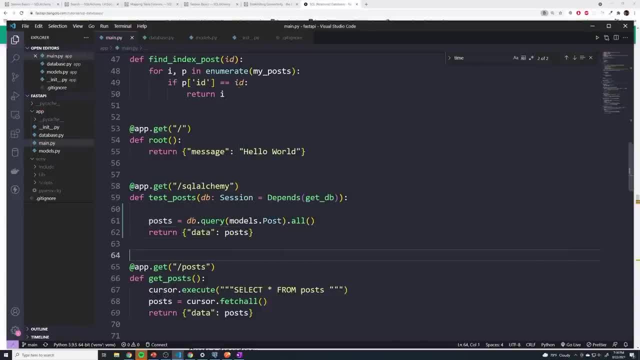 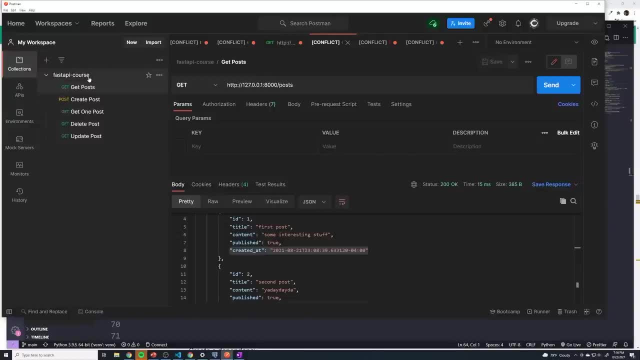 And then posts. So let's test this out now And I'm going to go to get posts. Actually, I'm just going to create a new test. test routes are a new request. I'm just going to copy the URL And then this is stored in SQL alchemy. Let's try this out And this should. 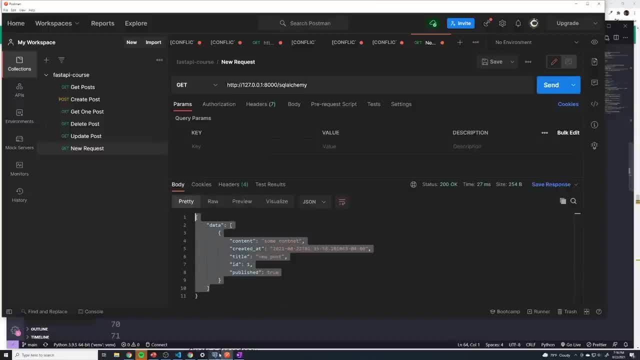 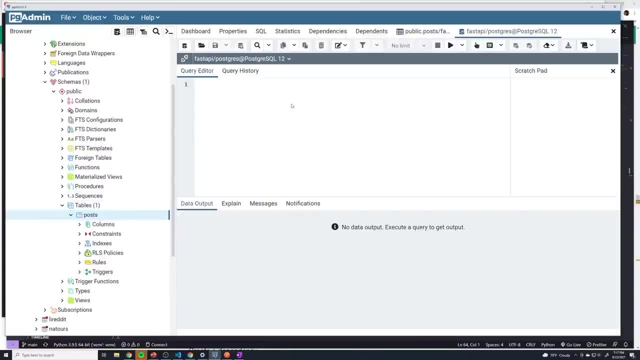 result in us getting just one post. So let me just double check my Postgres database just to make sure that we only have one post. So I'm just going to open up the query tool And we'll just use Select star from posts. 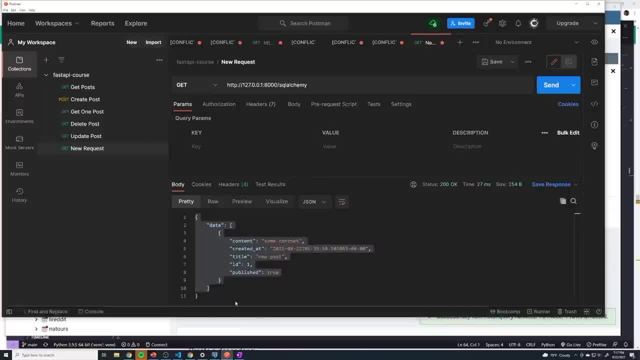 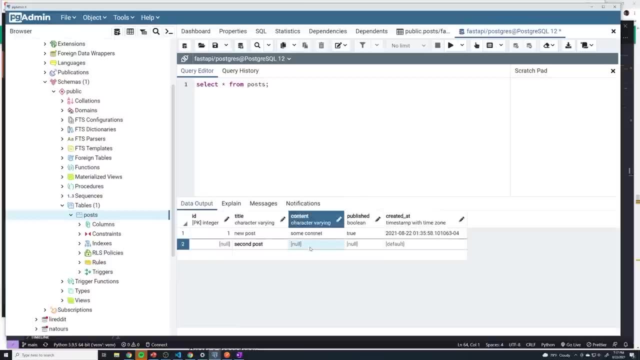 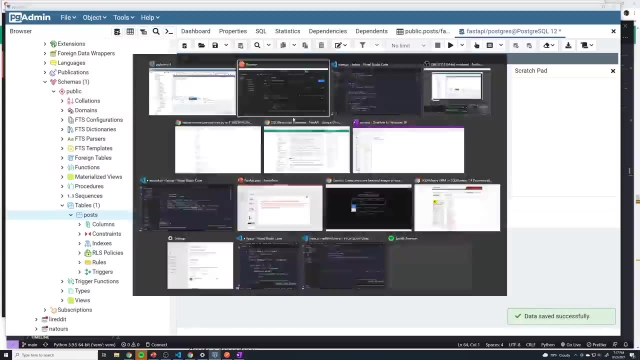 Yep, and it looks like I only have one post And so that's why we only got one post in our request request, And if I add a new post and save that and we make a new request, we should get two posts. So that verifies that we are successfully connecting to our database And 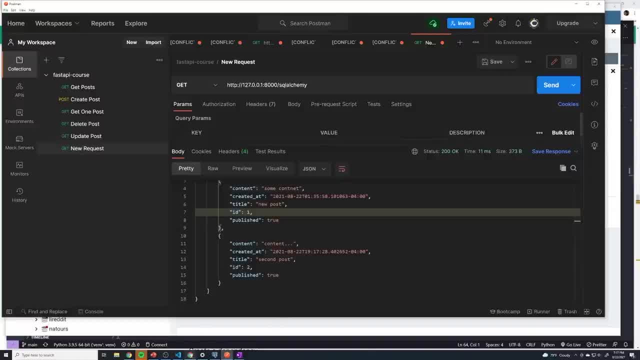 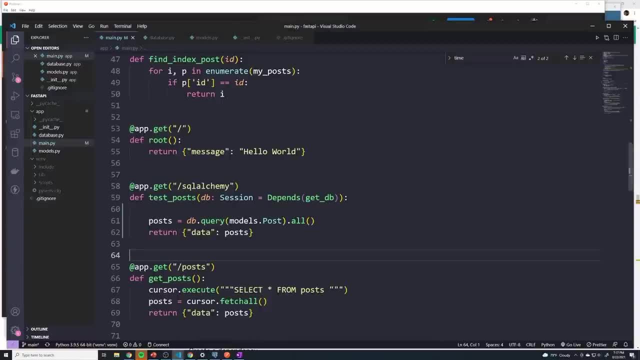 we are successfully retrieving those posts, And so I want you to stop and really take a look at how the queries vary when it comes to working with an ORM versus working with regular SQL, Because if we actually see the path operation for getting posts at slash, 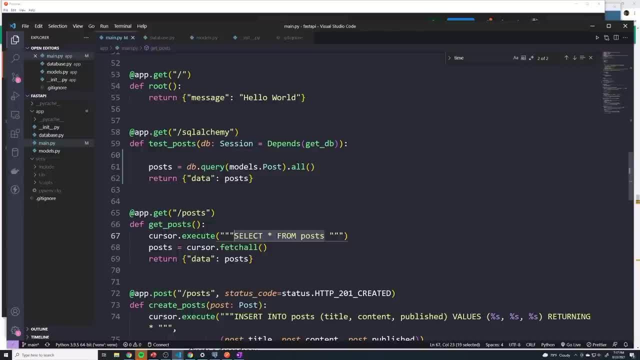 post here. this is where we're using regular SQL. So here we do select star from posts, But if you take a look at this, there's no SQL here, right? we're just tapping into the database object And we're going to call a query And then from here we have to tell. 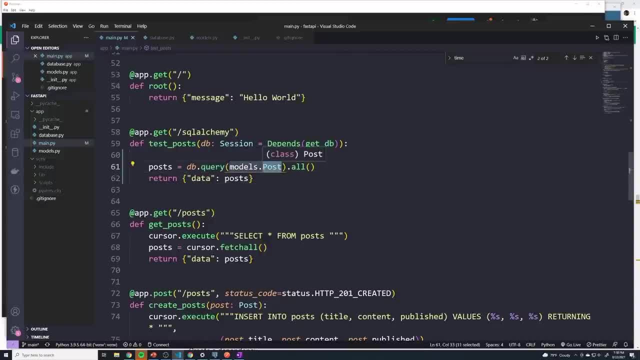 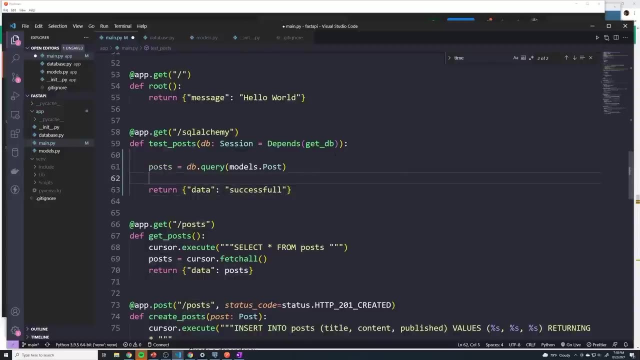 what specific model, which in this case, remember, these models represent tables, And then we just say: I want all posts. Now, what's even more interesting is if I remove this, and then, for now, I'm just going to hard code, you know, successful, just some random data. I'm going to do a print. 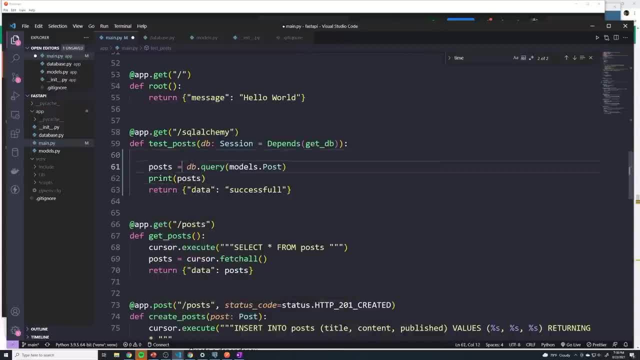 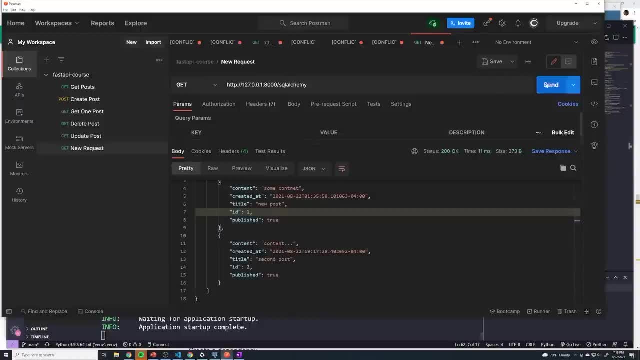 posts. So right here, we're calling the database object and then we're calling query. So what actually happens when we do do this? Well, I'm going to save that. we're going to send a request. we're not going to get any data back. that's to be expected, But take a look. 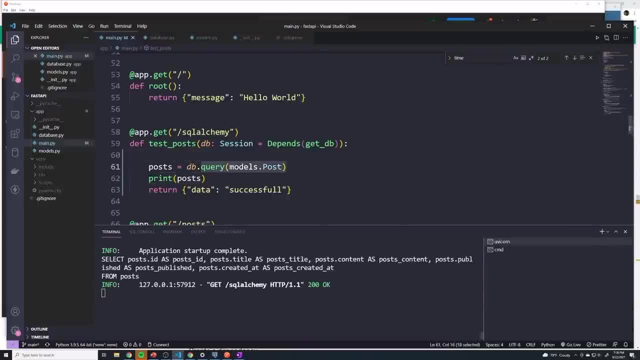 at this right. we're actually taking a look at what the query object returns And you can see that it's just returning a regular SQL statement. So it's saying I want you to return post that ID and then it's just renaming it: posts underscore ID. then I want to grab post that. 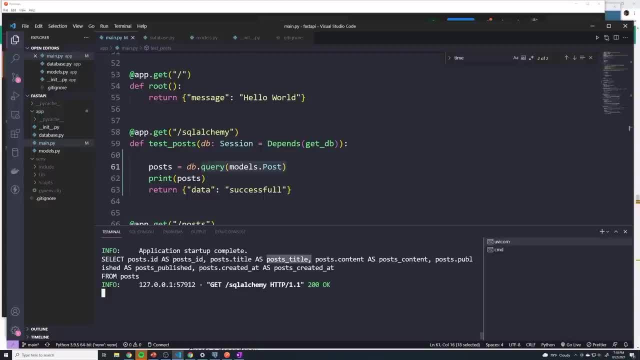 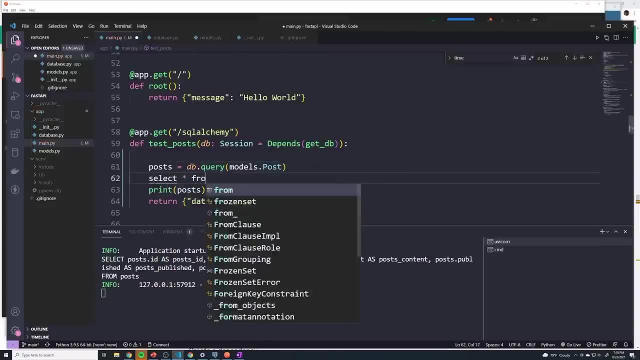 title. we're renaming it as post, that title, So it's grabbing all of the columns And then we're going to grab it from our post table. So it's really no different than just running. you know, select star from posts. essentially that's all it's doing, But it's just renaming. 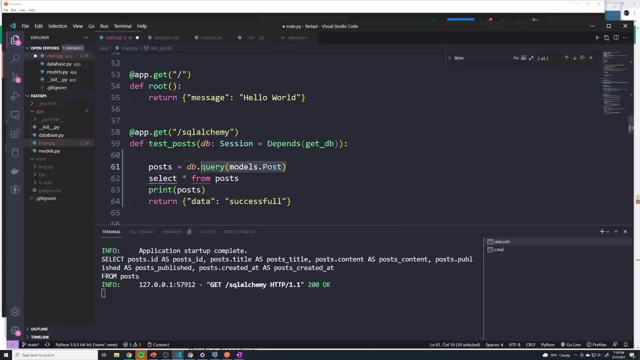 all the columns to be a little bit more easy to read, So you can see that these queries, this query object is just performing SQL, So it abstracts all of the SQL away from you And it handles all the logic of generating the SQL, so that you don't have to know, or 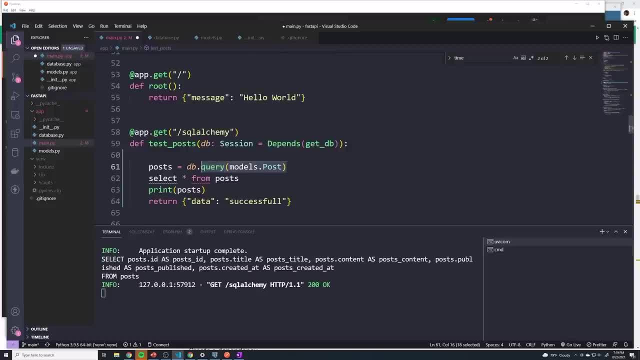 to have as solid of an understanding of SQL And this allows you to really focus on building out the API. This allows you to focus on working with Python and less with SQL and the databases themselves. So now we know. when we call query, this actually creates the query. However, to run the query, 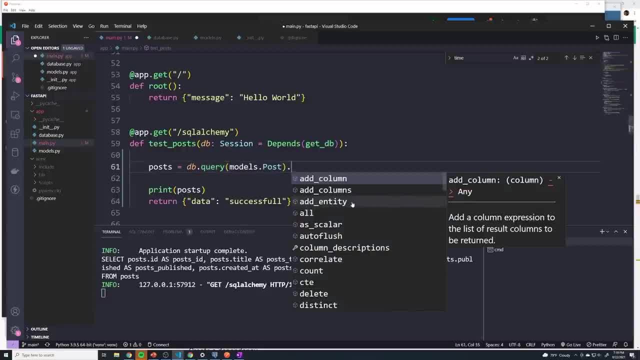 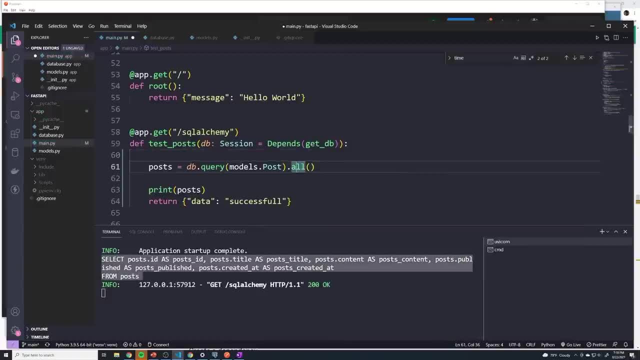 we have to run a specific method. So there's a couple of methods that we can run, But if you want to grab everything, then you just call all and then it's going to take this SQL query And then it's actually going to run it against the database and then return. 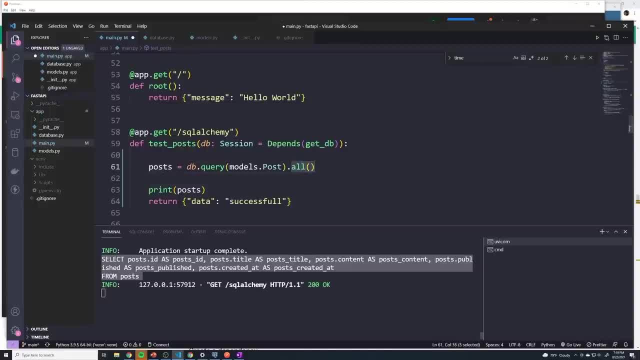 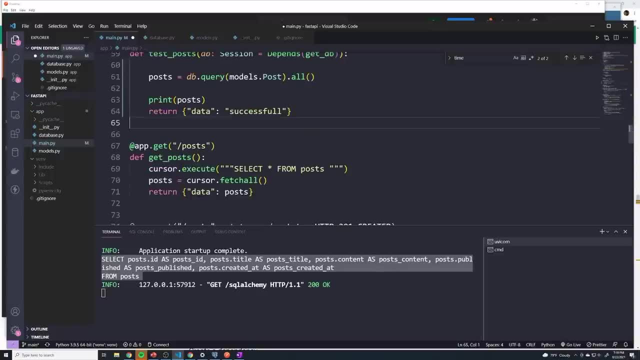 it. But until we call this last method, it's nothing more than just a SQL query that hasn't been run yet. Alright, so now that we know how to fetch all posts, let's just go down here Right and let's just put in this logic. So this is our actual endpoint for retrieving posts. 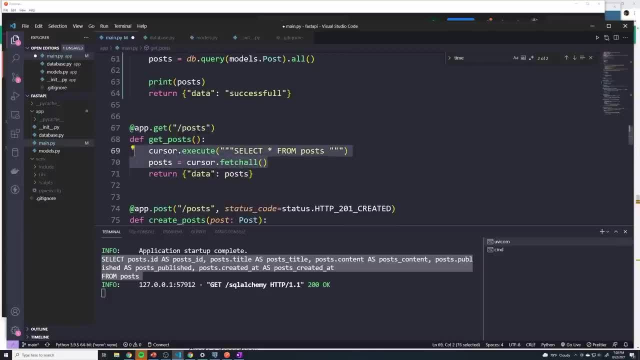 This is our get posts, And what we're going to do is- I'm going to comment this out just so that you know later down the road, if you guys want to just take a look back, how you do it with regular raw SQL. we still have that within the code base. 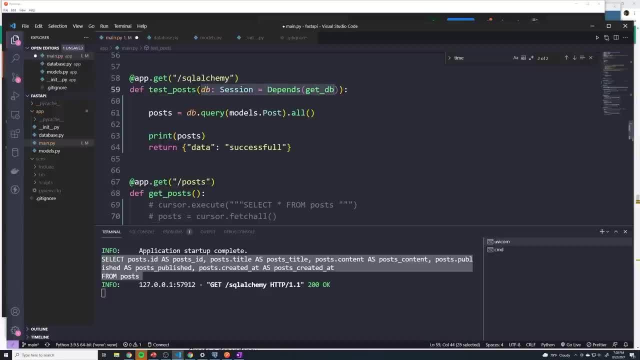 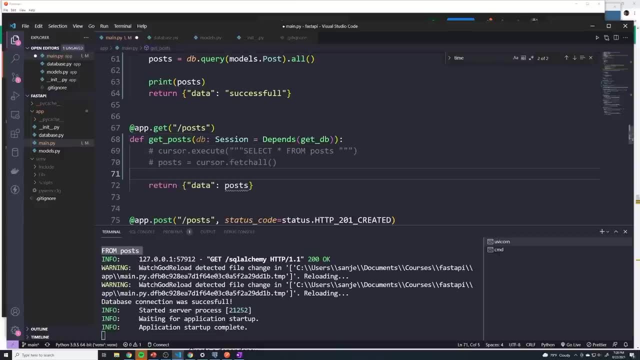 And anytime you want to work with the database, remember you have to pass it in to the path operation function. So this is going to make it a dependency And you'll see, by doing it like this, it'll make testing a lot easier. 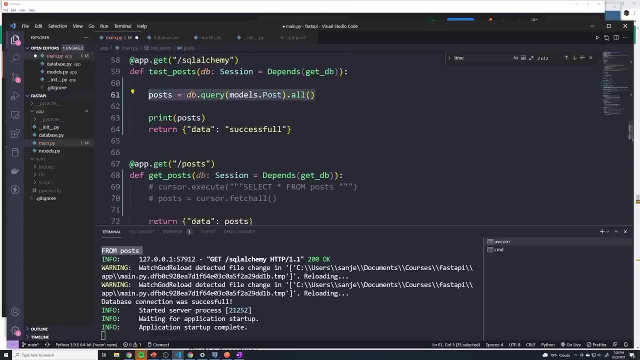 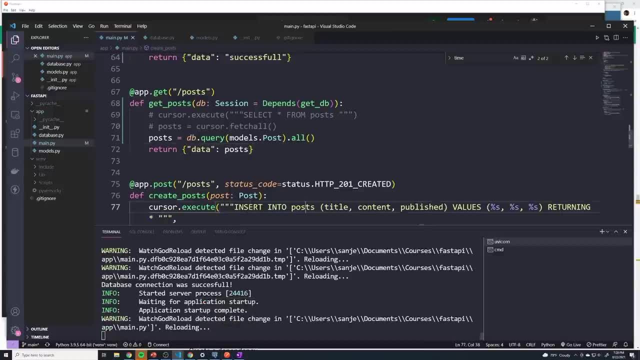 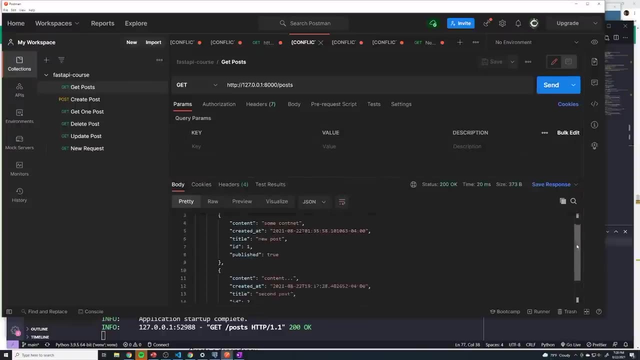 And then we can just copy this right here And then we're going to return the post. So let's test that out. And now, if I go to get posts hit, send, you can see that we successfully retrieved both of our posts. Alright, and it really is as simple as that. And then in the 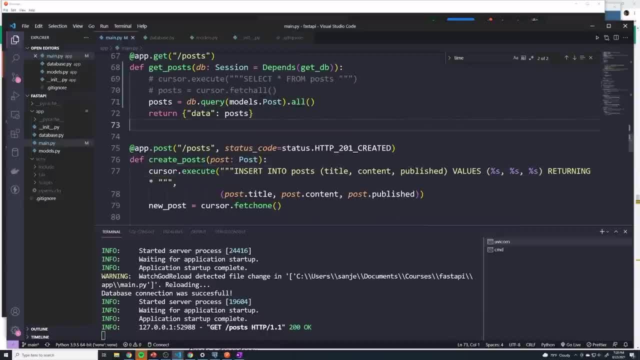 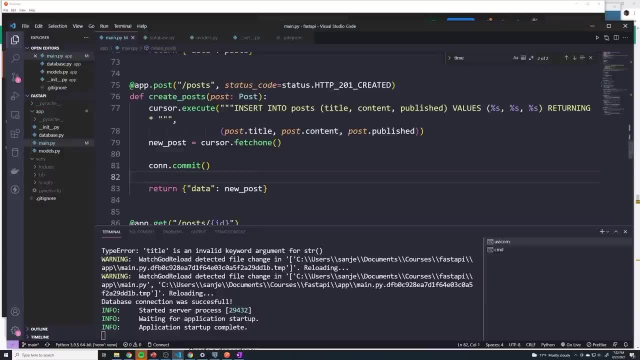 next video we'll start taking a look at how we can create posts and so on. In this video we're going to start tackling how to create a post using a ORM or, specifically, SQL alchemy. So once again, I'm going to copy out or comment out all of the SQL code. 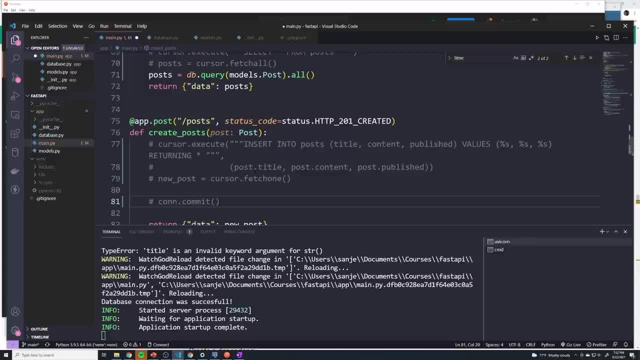 And what we're going to do is we're going to see how we can actually create a brand new object, or a brand new post in this case. So, first things first, anytime any of your path operations need to work with the database, we need to make sure that we copy this exact input argument into the path. 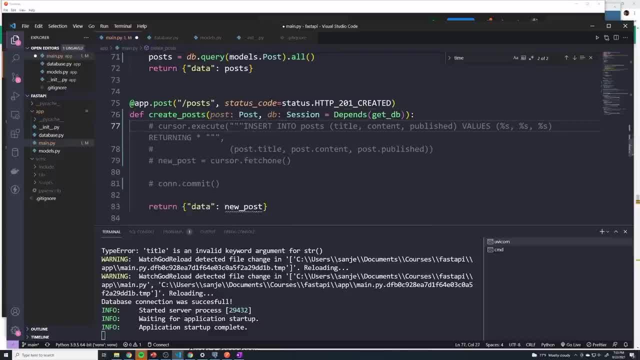 operation function. This is going to give us a access to our database object so that we can actually make queries and make changes to our database, And by passing it in like this, it's going to make it a dependency and it's going to make it a lot easier for testing and and things. 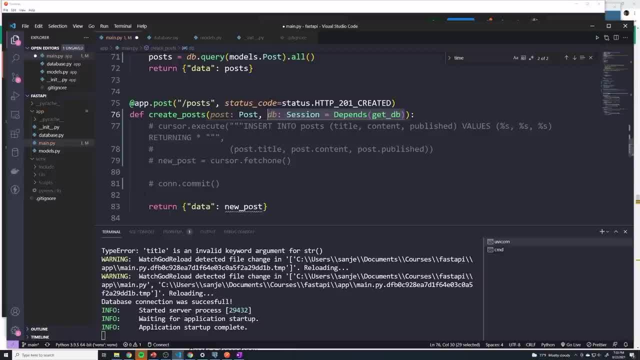 like that. Technically, you don't have to do it like this. You could just import it directly in there. However, by doing it like this, like I said, testing becomes a little bit easier. Alright, so we've got our models right and we have. 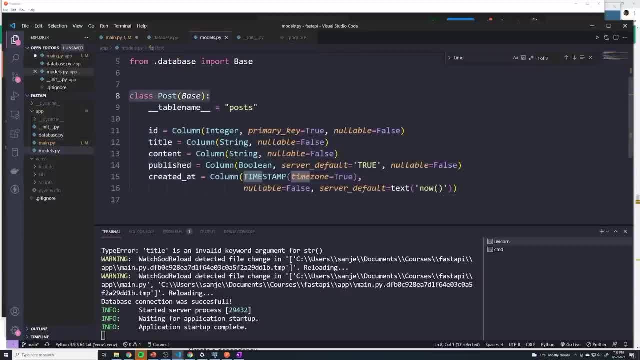 one specific model. So this model represents our posts, And so to create a brand new post, we have to reference this model and pass in the specific fields that we want to create a new entry with. So first of all, we have to make sure we import that model, And you can see that we are. 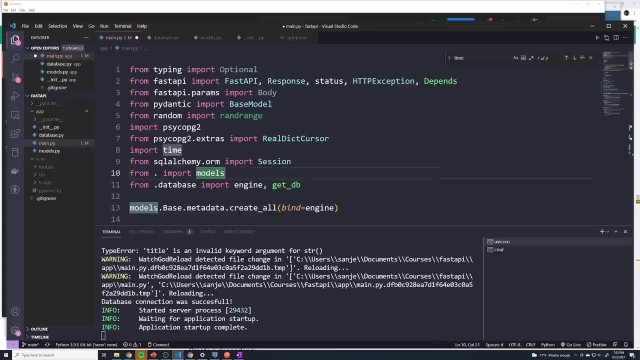 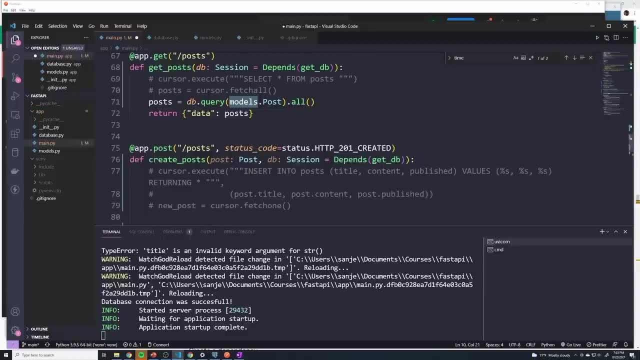 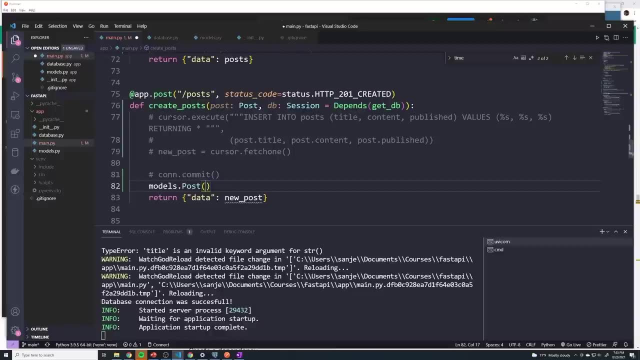 importing all of our models by doing from dot import model so we can access models dot post, in this case to X, that specific model. And so here I'm going to do models dot post, And then we have to pass in the properties of the brand new post that we want to. 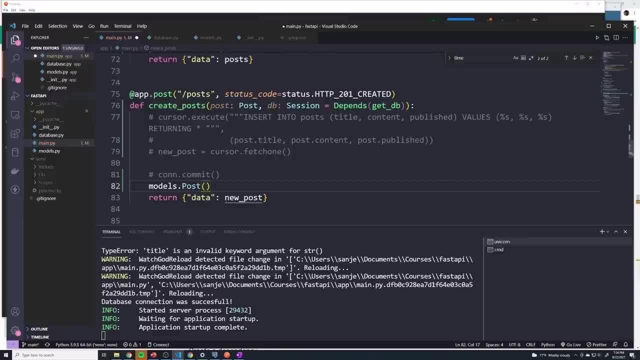 create. And so what are the properties right? If you take a look at our SQL statement, we need the title, the content and the published Boolean right, and that's all going to be derived from the request that we get, which is going to be stored in the post object: So I can reference: 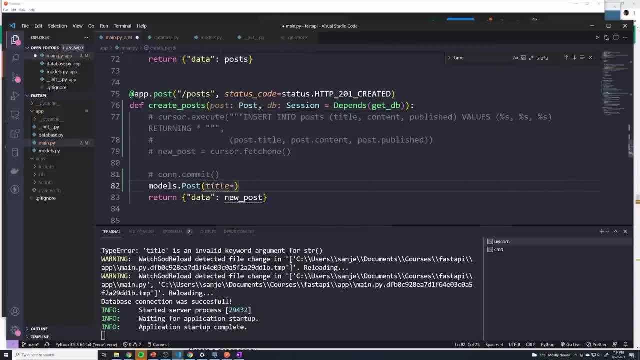 all of those fields. So I can say the title for the brand new post is going to be set to. whatever the title, the user center and that can be accessed with post dot title, the content of the brand new new created post is going to be: content equals post dot content, And then the same thing. 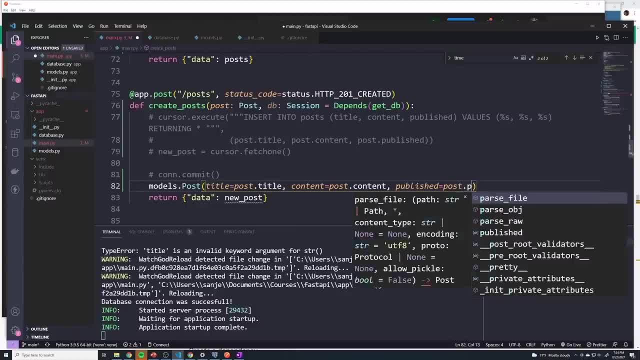 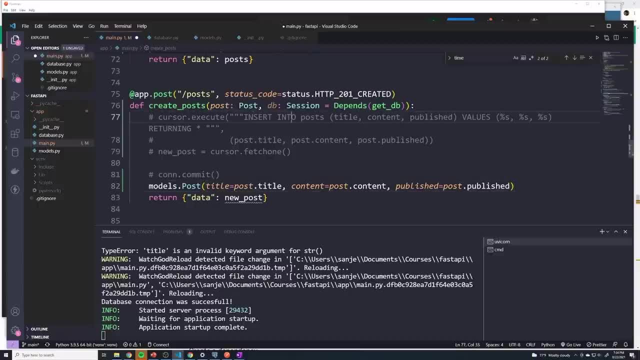 is going to be for published, So it's going to be post dot published. And if you take a look at this code so far this doesn't look too different from the SQL statement, right? This says insert into posts and then we pass in: post that title into the title, post content into the content. 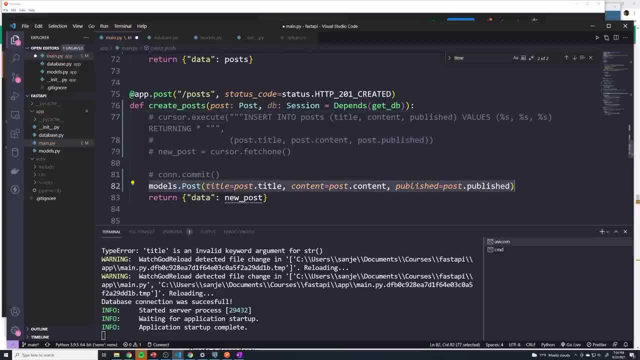 and then post that published into published right, And so this is pretty much exactly the same thing. We're not doing anything different, We're just having SQL alchemy handle all that logic, So we can do everything in just standard Python code And there's no sequel anymore. All right, And. 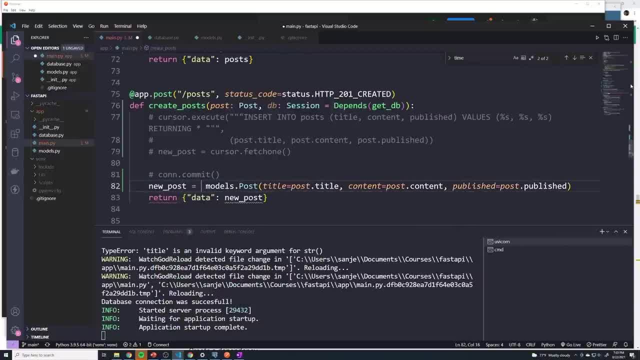 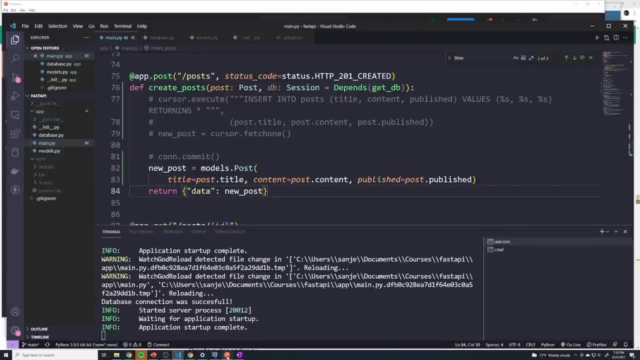 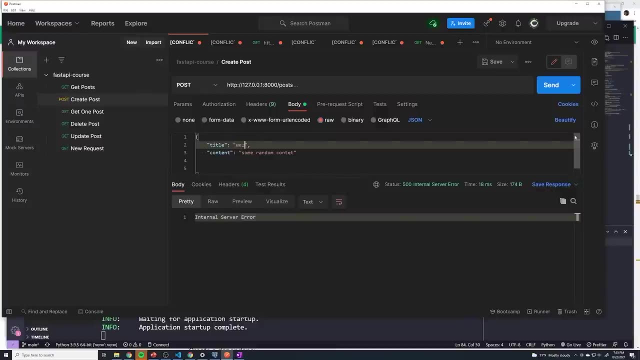 the next thing that we want to do is, well, let's save the result as new post And let's see what happens. So I'm going to save this, And then we're going to set a little query. So, first of all, I'm going to create a new post. I'm gonna call this a welcome to funland. 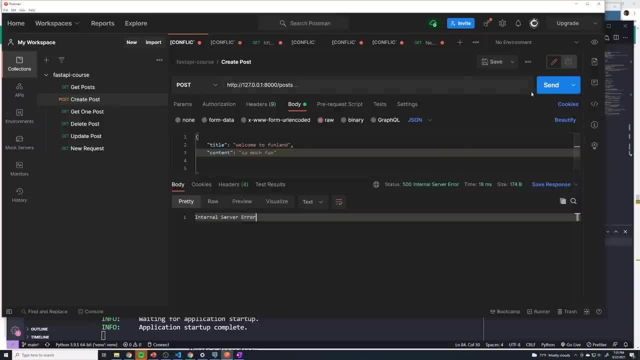 So much fun, Okay, and so then we'll, we will send a request And we got some data back, And so it looks like it worked. However, take a look at our, our data. we've got a title, we've got a content and then we've got published, but where's the ID, Where's the created ad? 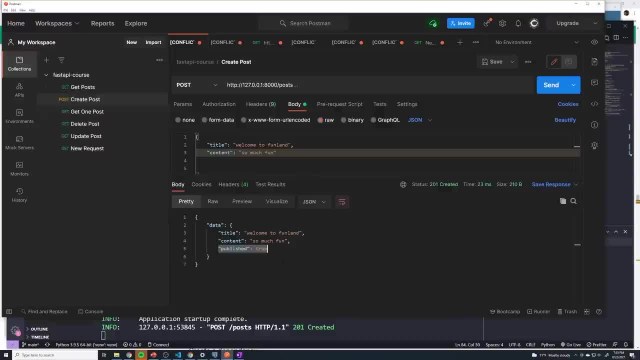 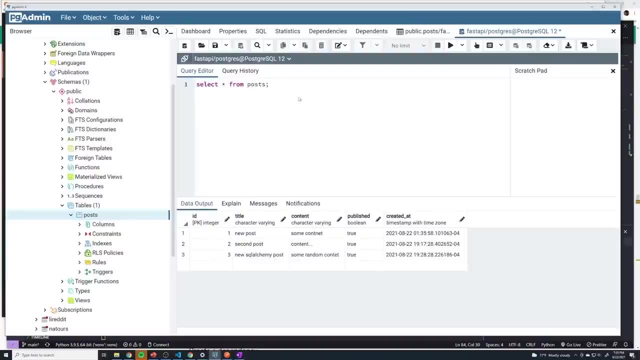 field, all the fields that the database creates. So this makes me suspect that this didn't actually work. So let's go to Postgres And go ahead and make a query to your table. So select star from post. that's going to grab all of them And you'll see that based 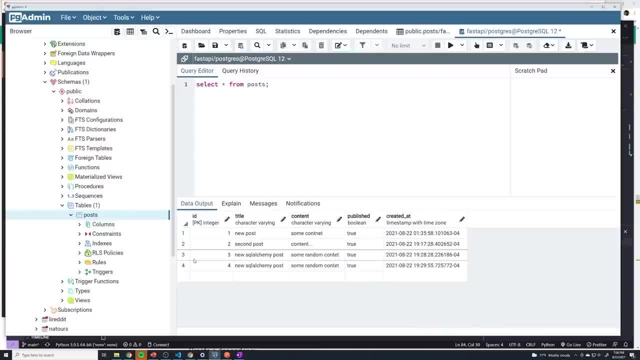 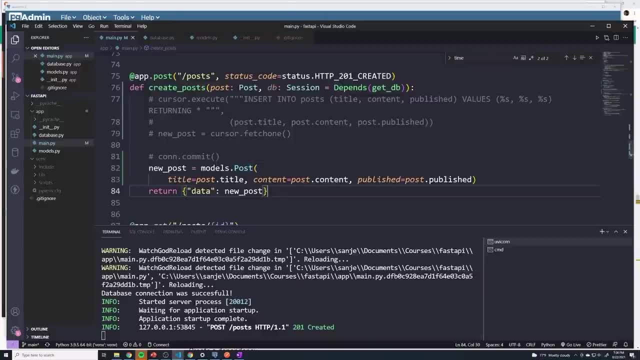 off of the title: welcome to fun land. I do not have that in there, So it looks like this was not successfully able to create a post within our database. So let's take a look and see what went wrong And if you actually take a look at the, the previous method right. 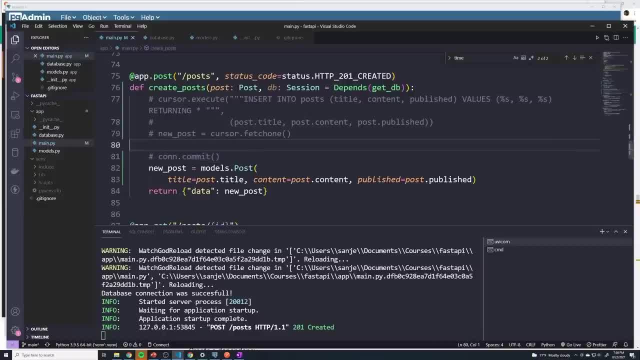 you could see that we actually have to commit something to the database So we can create an entry, but it doesn't actually get pushed to the database until we do a commit, And so I'm suspecting that we probably have to do a similar thing. So 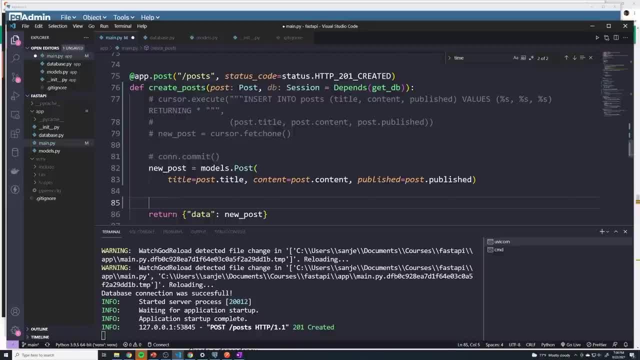 when it comes to SQL alchemy, what we need to do is, first of all, you have to tap into the database object. Now we want to say db dot add, and then we're going to add this newly created post, So this is going to add it to the database. However, just like with 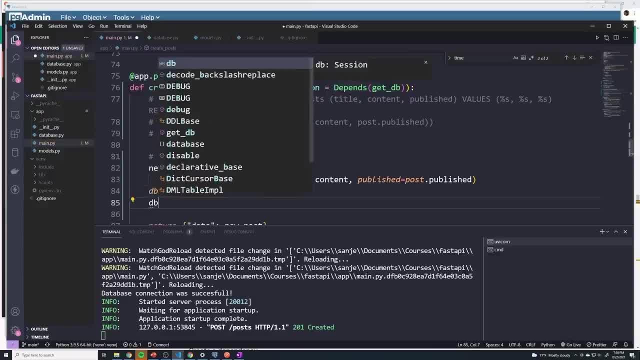 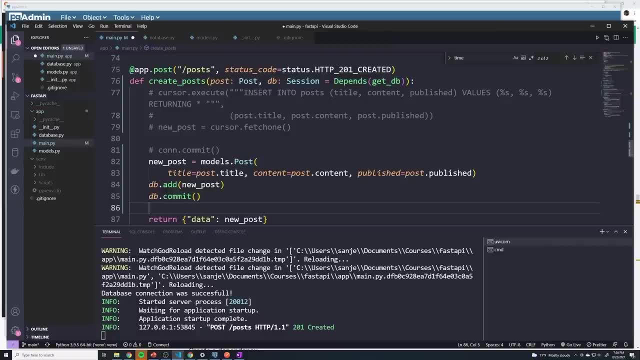 the connection dot commit. we have to commit those changes. So we do db dot commit. And then the last thing that we need to do is, if you take a look at our SQL statement, we have this returning star. So that's going to return back the newly created post With: 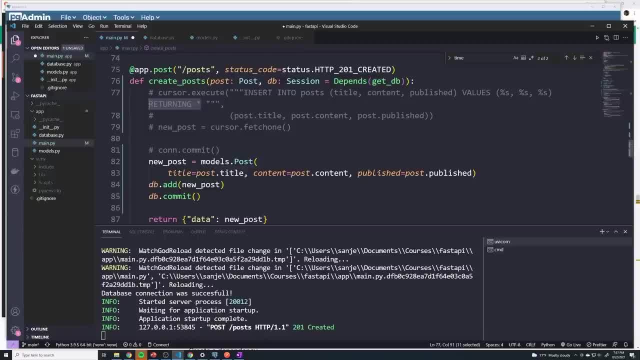 SQL alchemy it's a little bit different, right, Because we don't really have access to that underlying SQL code. we can't add a returning statement to this. So the way that you do this in SQL alchemy is you do db dot refresh And then you pass in the new. 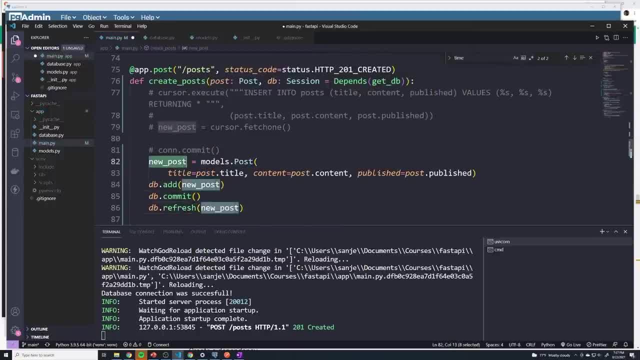 post object. So what this is going to do is we create a brand new post, we add it to our database, then we commit it, And then what we're gonna do is we're going to essentially retrieve that new post that we just created and store it back into the variable new underscore. 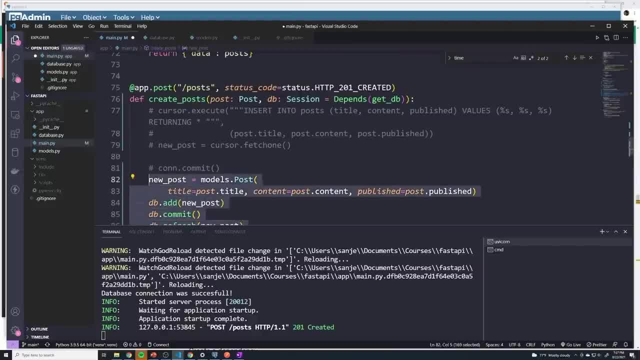 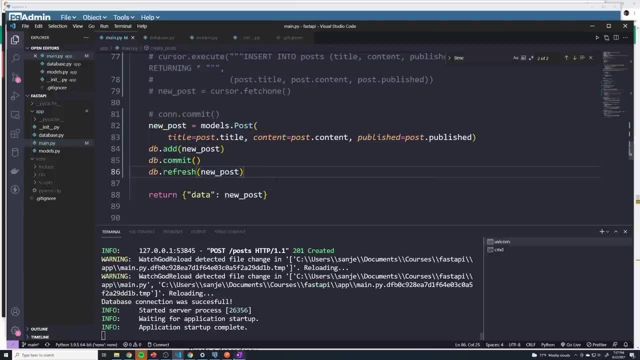 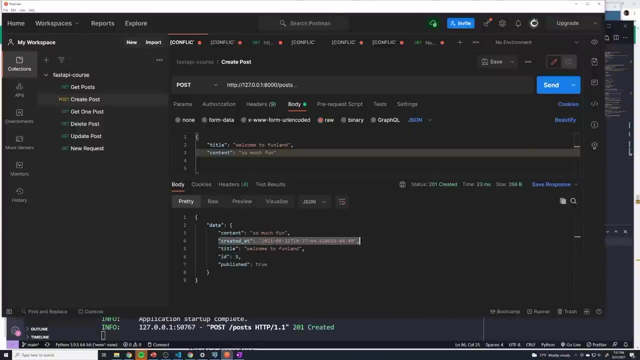 post, And so all of this code should be identical to this code. And so now, if we will just return back new post, and I think that should fix our issue- So now, if I hit send, we do see an ID and we do see a created, I feel. so it looks like it worked, but we want to double. 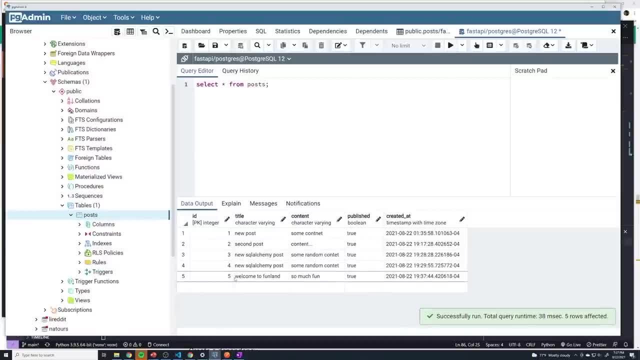 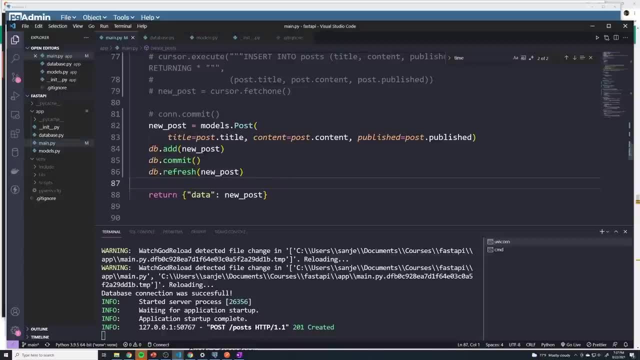 check within Postgres. So if I hit run and we can see: Welcome to Funland. So it looks like it's now successfully working. And before we wrap up this video, there's one thing I don't like about the way we've done things right, And this isn't necessarily going to break or cause any issues. However, 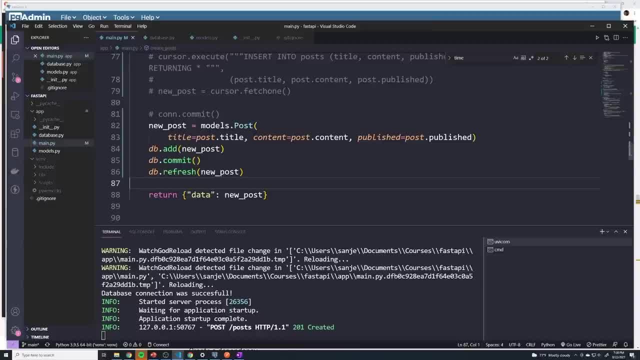 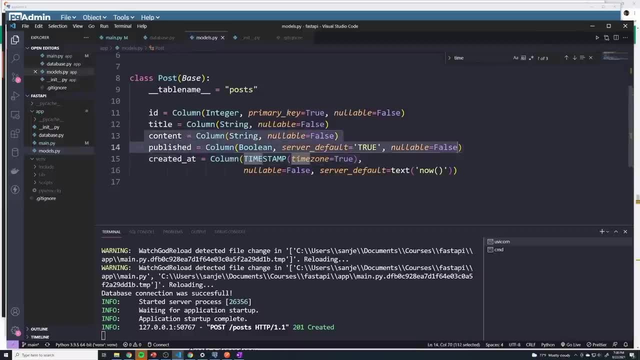 you're going to see it's very inefficient, depending on what your models look like Now, our model has only a couple of fields and the user only has to really pass in two to three fields, which is title, content and published. So it's not that big of a deal, But imagine, 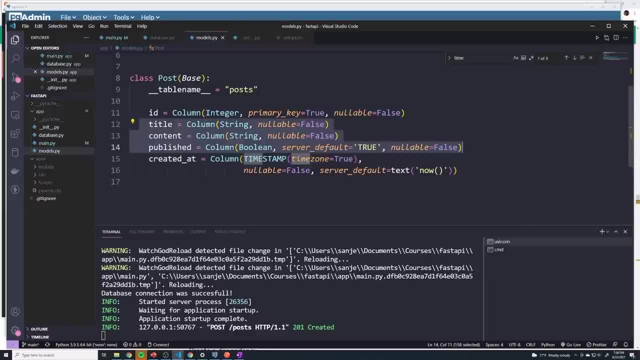 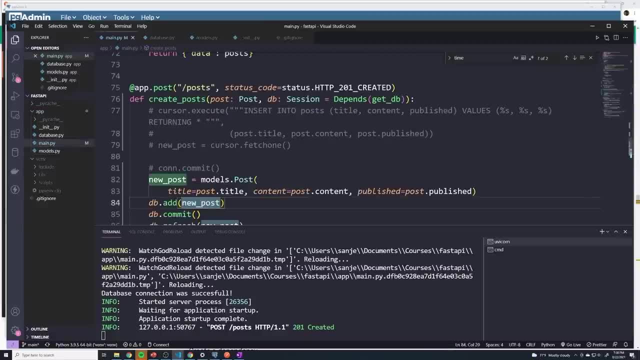 if we have a model with 50 fields- there's no limitation, right? You can put as many fields as you want- well, then things are gonna get a little bit more difficult, Because if you see, we have to extract all the fields from our schema, right, and then we have to kind of pass it into, we have 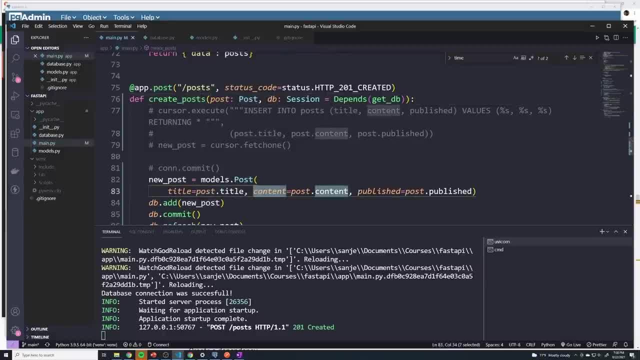 to say, Oh, title equals post, title, content equals post content, and then published equals post published. Now, if we have 50 fields, we're gonna have to do that 50 times And that's a little inefficient And there's actually a much easier way to do it And the way to. 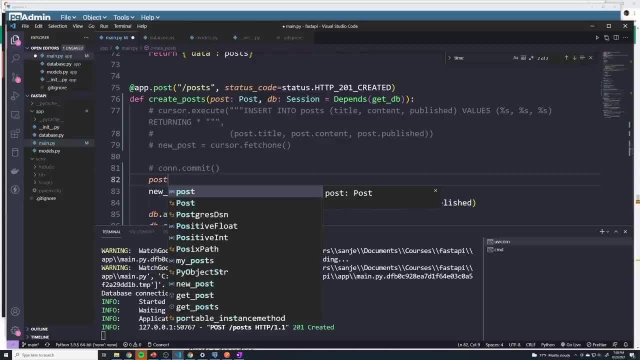 do this is we have access to the post object, which is, you know, this is a pydantic model, So it's going to ensure that it matches the schema that we set And we want to say post dot dict. Now we know that's going to. 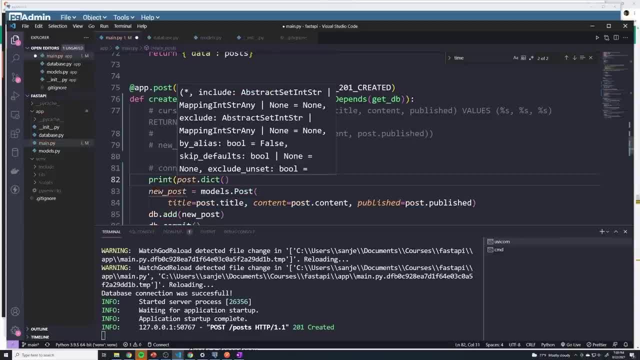 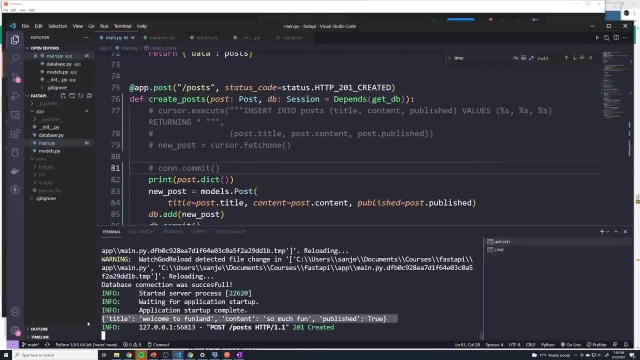 convert it to a regular dictionary. So if I do a print, save that and then just send a request. right, take a look at this. we've got a regular Python dictionary. However, we need to be able to automatically take that dictionary and convert it to this format, where 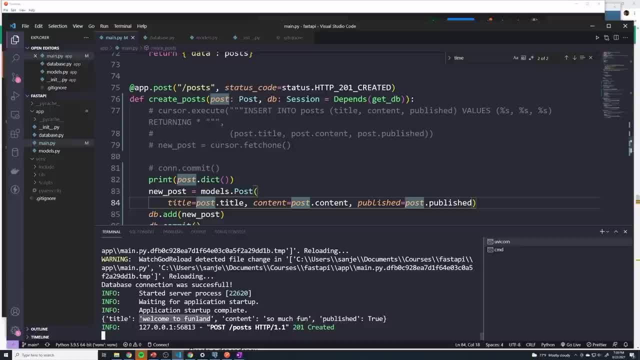 instead of having you know title like this, we're going to be able to convert it to a document like this and then welcome to funland. it's going to be title equals and then post out: title content equals post content. So how do we do that? Easy, all we have to do. 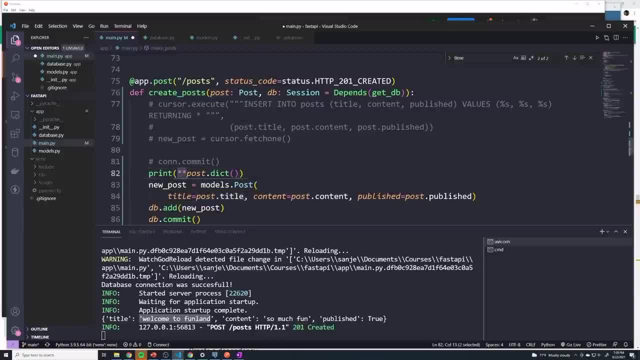 is: unpack the dictionary, So you just do a star- star and it's going to put it into this exact same format. So we can remove all of this And just say star star, post dot dict. And that should ultimately do the same exact thing, Except now if we go back to our database. or our model and add an extra fields, it's going to automatically unpack the dictionary And that should automatically do the same exact thing. Except now, if we go back to our database or our model and add an extra fields, it's going to automatically unpack. 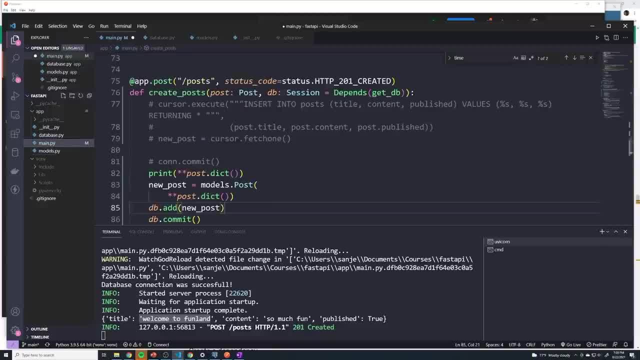 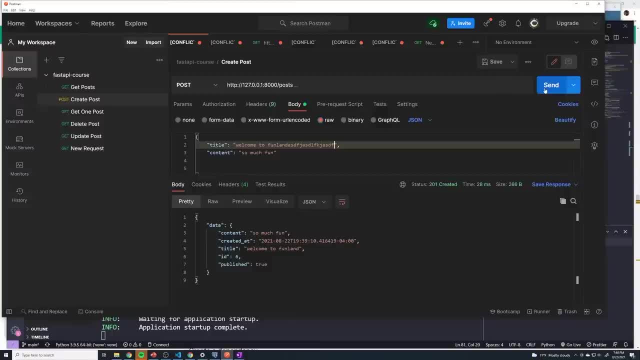 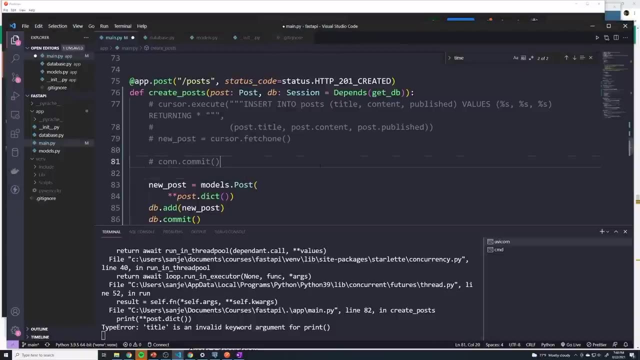 all of those fields for us, So we don't have to manually type it out. I will save that. I'm going to just put in some extra text just to make sure we can verify that. And I realized we got to remove this print statement and throw an error And we'll hit send. it looks. 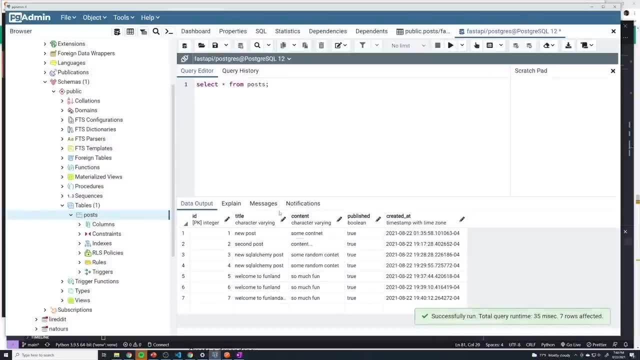 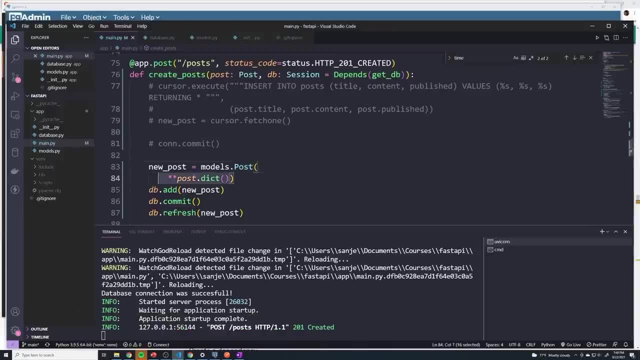 like everything worked. Let's go to our database search and it looks like it worked. So you can see that if we go back to our code, a lot cleaner than having to type out each one of those fields And we can put this: 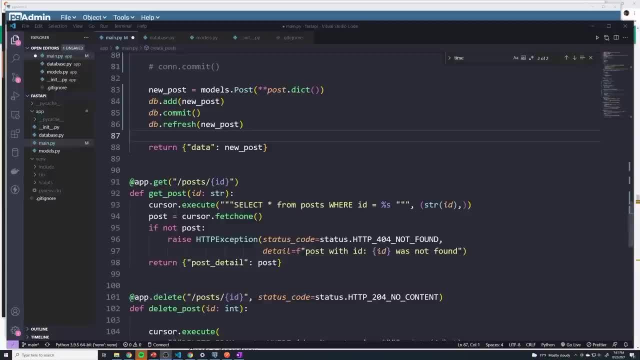 all in one line, So it looks a little better. Alright, so now it's time to handle querying for an individual post. So I post by a specific ID. So once again, we will comment out the SQL code And we will do this using SQL alchemy. 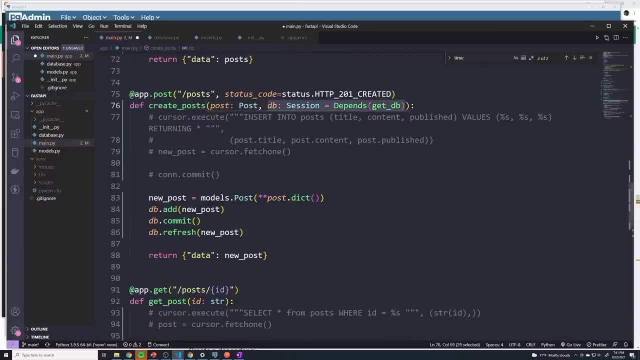 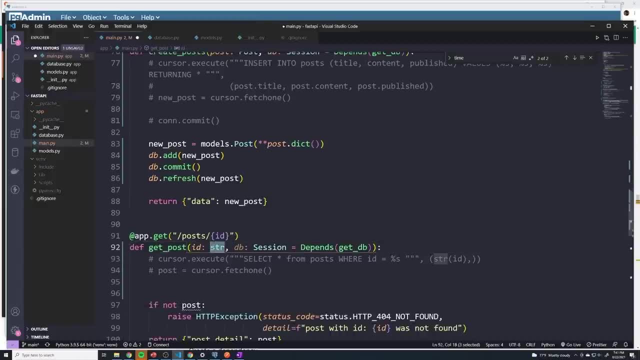 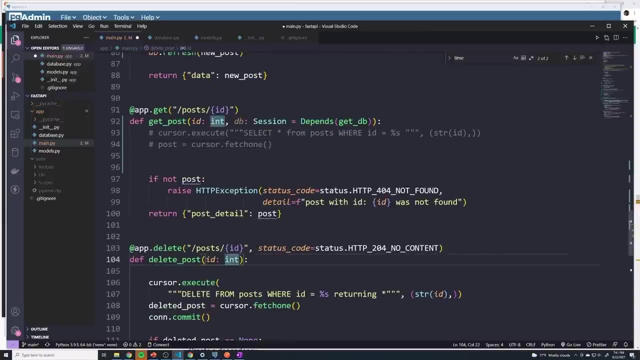 So, once again, copy the database dependency right here and then just pass it in. And this should actually be an integer. I don't know who changed that. I may have left that in from the previous video. Yeah, it should be an integer. Okay, And now what we want. 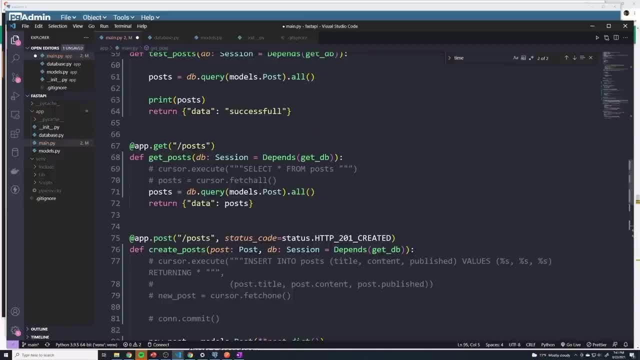 to do is just like we saw when it comes to querying all posts. we have to do DB dot query pass in the specific model that we're interested in, And then we're not going to do a dot all because we don't want all the posts. So we're gonna have to take a look. 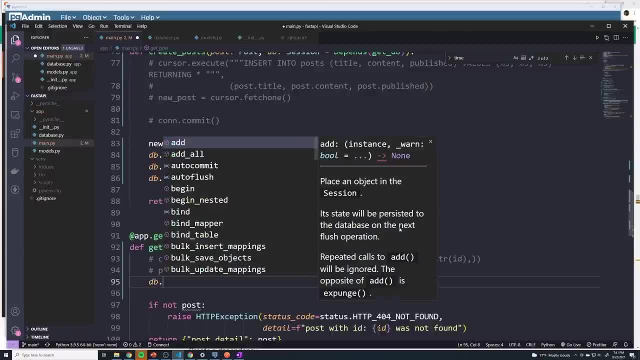 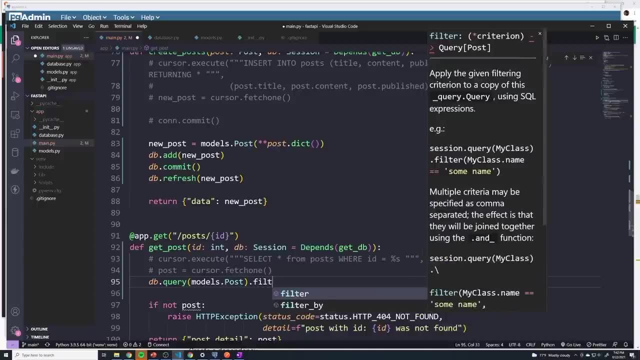 at a different query operation. So I'll say DB dot query Models dot post. And then we want to filter, So we want to pass in a filter. So this is the equivalent of doing like a, where you can see that we filter by doing where ID equals. 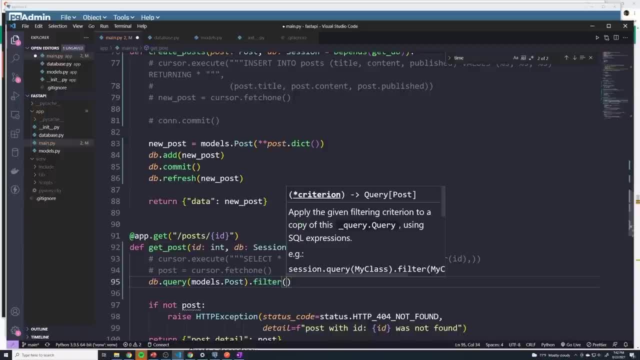 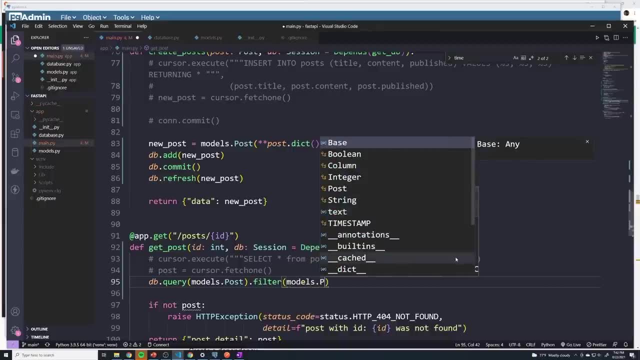 and then we pass in the ID. In this case we're going to filter And then here we say, whatever the models, dot, post, dot ID is. so this is going to look through all of the posts in our database And it's going to take a look at all their IDs And we want to see 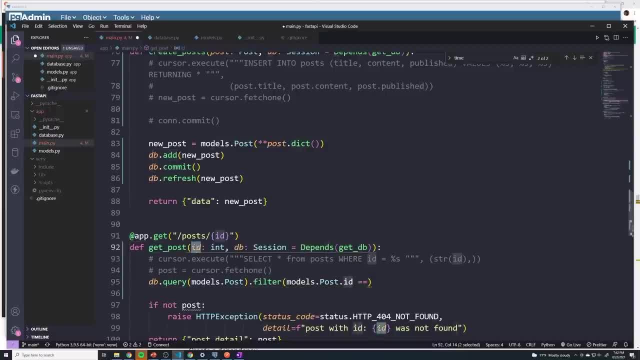 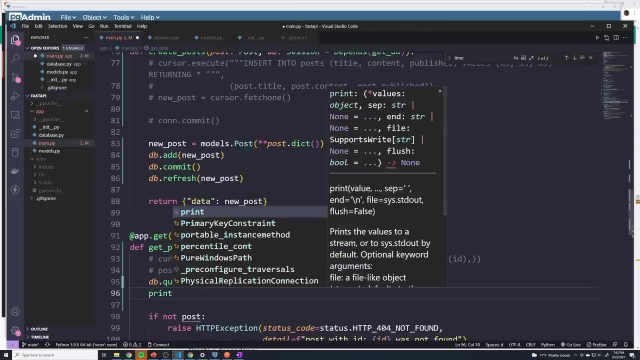 whenever that is equal to the ID that the user requested, So the ID from this query parameter or this path parameter. So we say, when they're equal, that's the one we want to return. And if I do a print of first of all, let's save this to a variable, So I'll say post equals And I do a print. 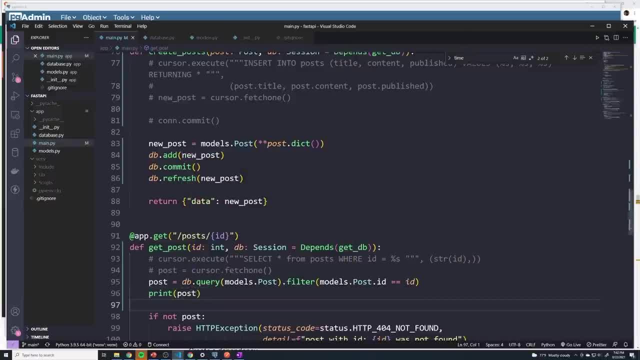 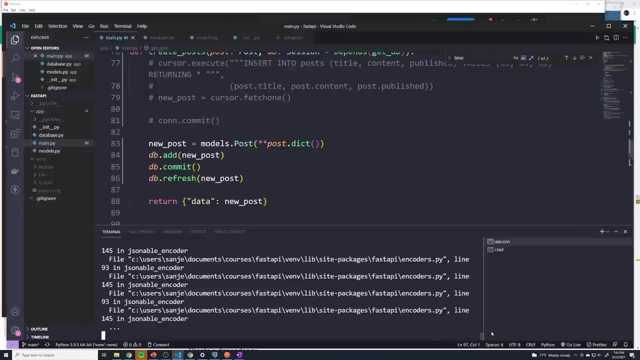 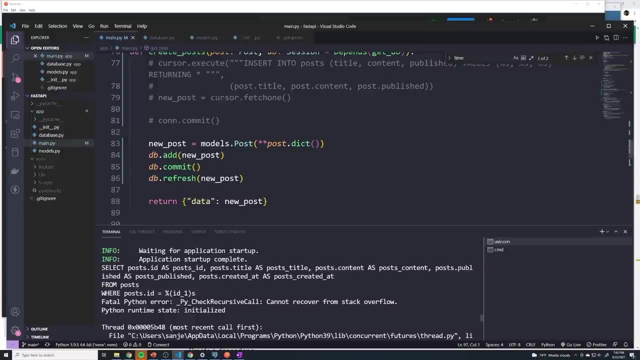 of post. Save that. I'll open up the terminal And then we'll send a request for an individual post And then we'll click send. We get a whole bunch of errors. That's okay, Let me see, And that's fully expected, All right. and then we can see the exact SQL statement that. 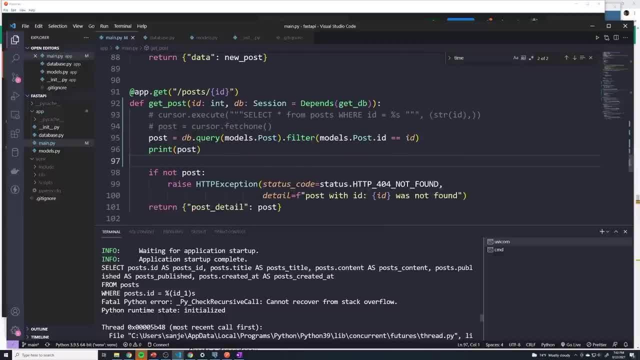 this query actually made. And so here we're doing DB dot query and then filter and we can see that we got the select statement And then here it's just grabbing all of the all of the columns, Right, but then you can see from posts and then it says where post. 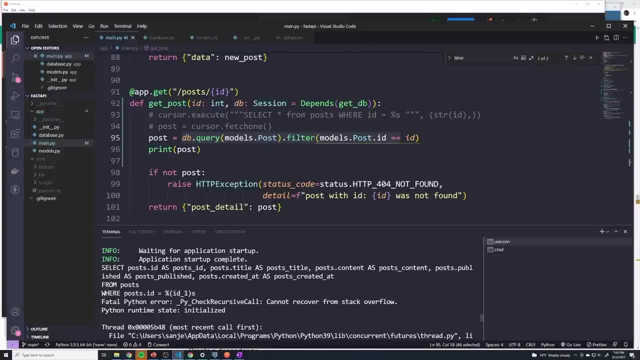 that ID equals ID underscore one, And so this pretty much looks exactly how like we wanted, right? If you look at our SQL statement originally, it doesn't look any different, And so at this point, I think this should be good to go. However, right now it's still just raw SQL. 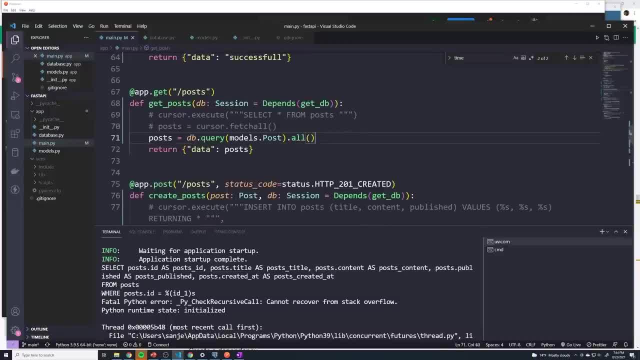 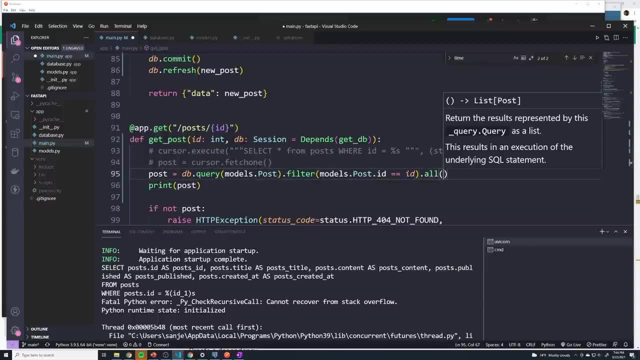 right, We could see what the SQL statement is. But if you recall from the previous one, we had to do a dot all to actually send the query. So for us we can do a dot all technically And this would work right. It would grab all of the columns, Right. This is just a. 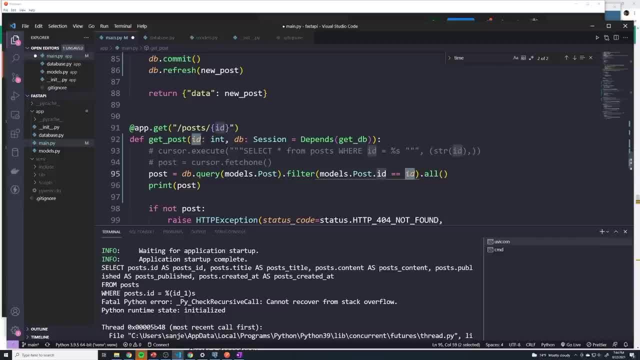 simple way to do it. It would grab all the posts who have an ID, of whatever ID we passed in. However, there's one little issue with doing it like this, And that is that once it finds one post, it's going to keep looking through all the posts to see if there's any. 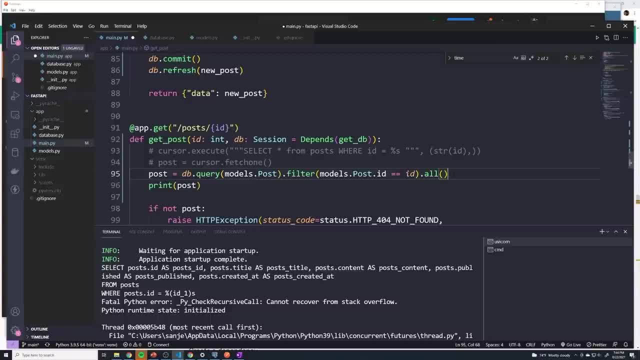 other ones, But we know that only one post can have this specific ID, So it's a waste of Postgres resources to continue looking when we know there should only be one. So, anytime you know there should only be one, instead of doing a dot all is better to do. 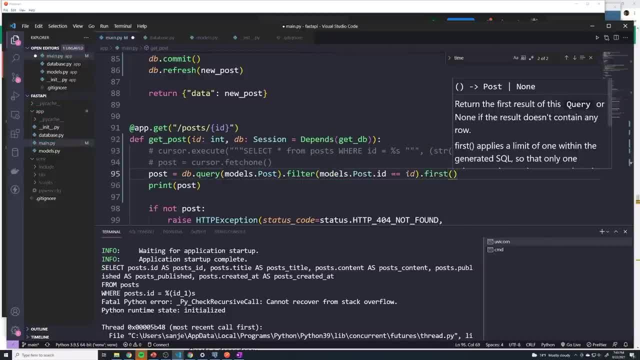 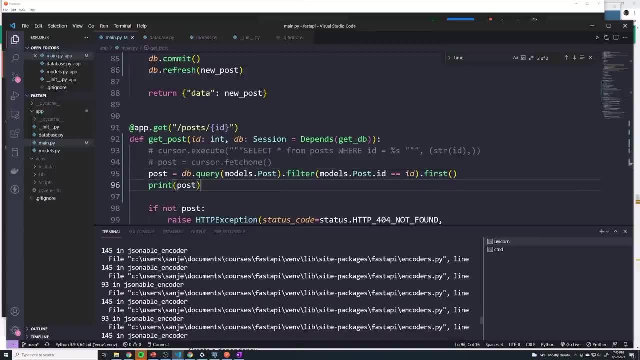 a dot first, So it's going to find the first instance and going to return that, so it's going to save us some of the time. it's going to be a little bit more efficient in that case. Alright, let's save this And let's try this again And let's see if this works. 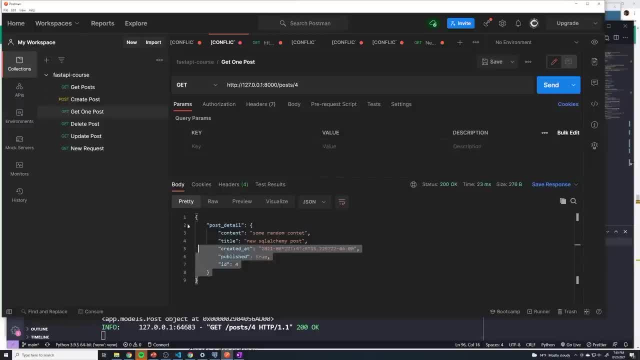 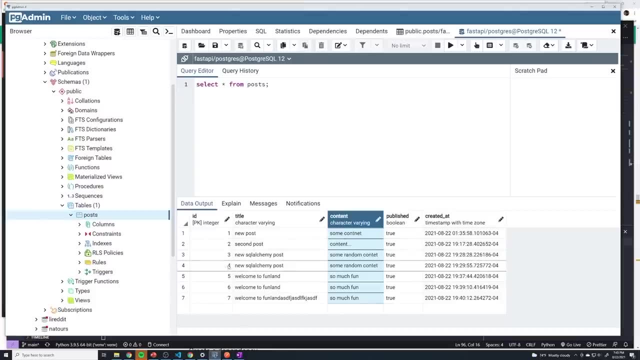 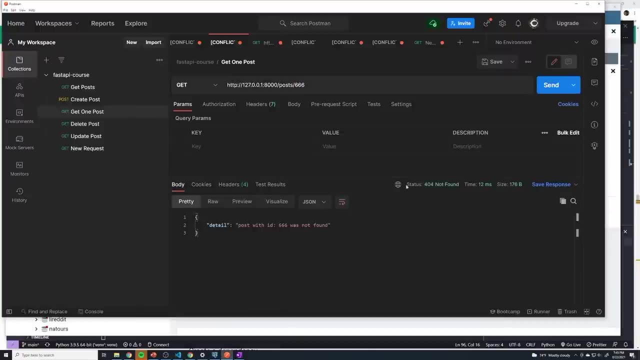 Alright, it looks like it worked. We got a post back, No errors, So I think everything is good to go. Let's go back to our Postgres database. we do see that there's one with an ID of four, So it seems to work. But let's test this out with a random ID of like 666.. 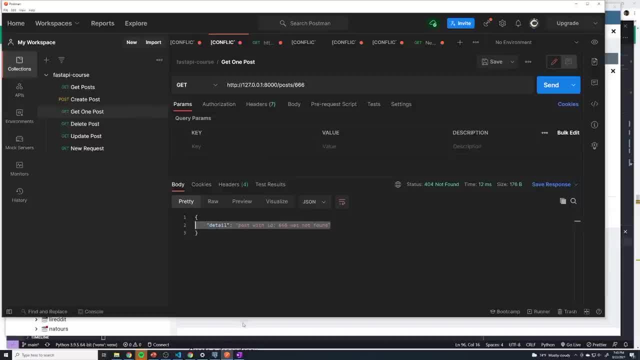 And we should get the 404.. So looks like this is going to be a good idea, And we can see that we're going to do it here, And here's what we're going to do here. So I've got a, So looks like that's all we need to do when it comes to fetching an individual post. 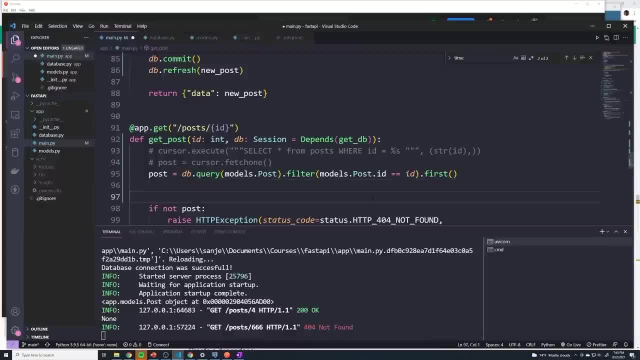 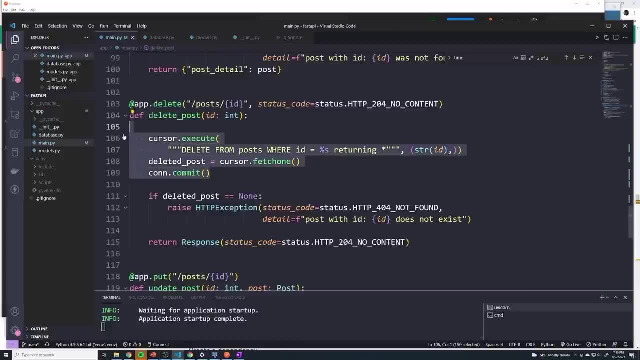 And I'll remove this print statement. we don't need that anymore, And then we can just conclude this video. Alright, so let's move on to handling our delete path operation. So I will comment out the SQL code once again, And then we're going to make sure that we pass in. 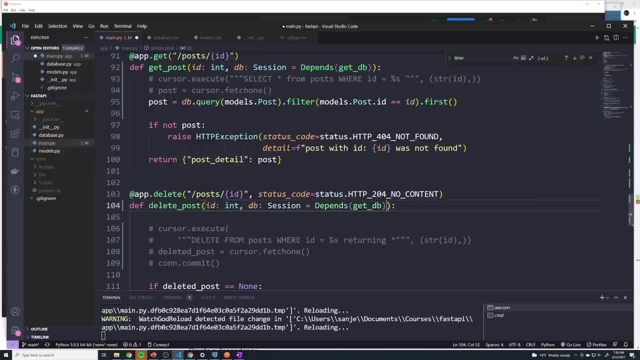 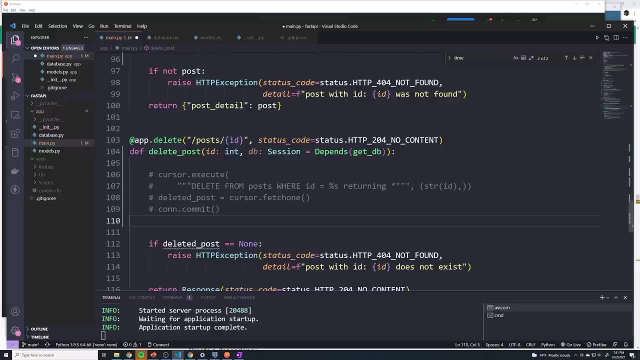 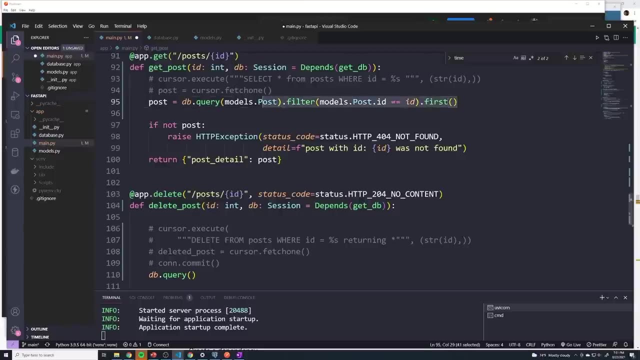 the database dependency into our path operation function And so, for our delete operation, what we're going to do is I'm going to do a query And this query is going to look exactly like this query, So I can actually copy this one in this. 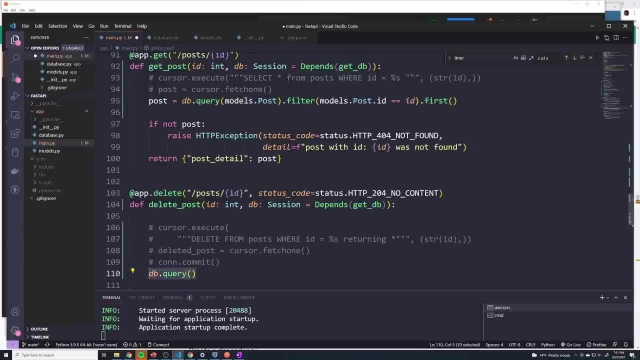 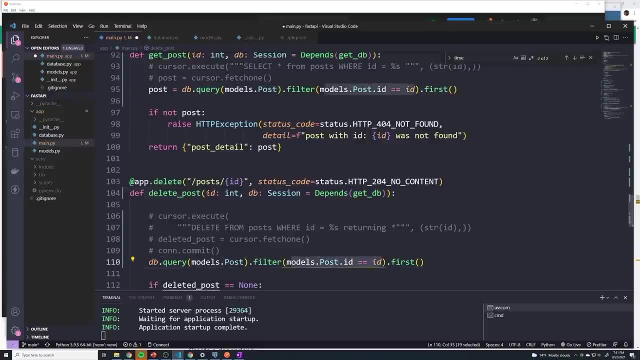 case. So all we're doing is we're grabbing the posts model And then we're going to filter based off IDs. we're going to look for the ID of the post that we want to delete, And I'm actually going to remove this first. So I'm going to save this as a post And then I'm going to save this. 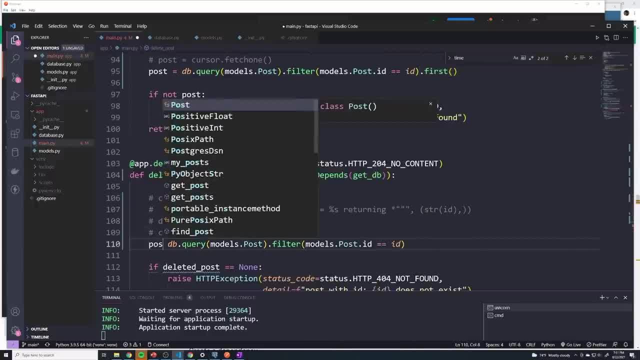 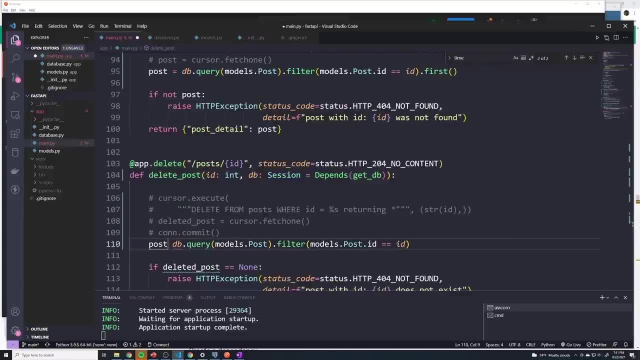 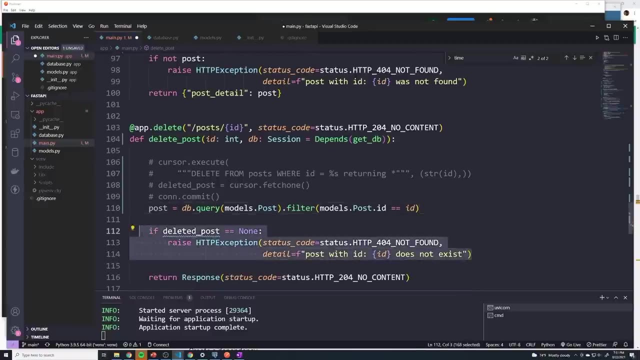 save the query by itself And we'll save this as a post underscore query. I'll just save it as post. Okay, we'll understand that that's a query and not an actual post. And then our if statement to check if there actually is a post with that. what we're going. 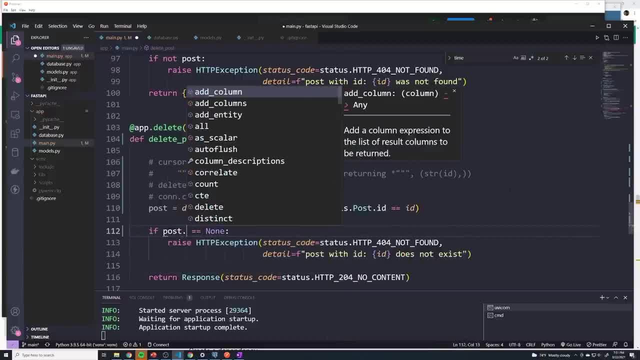 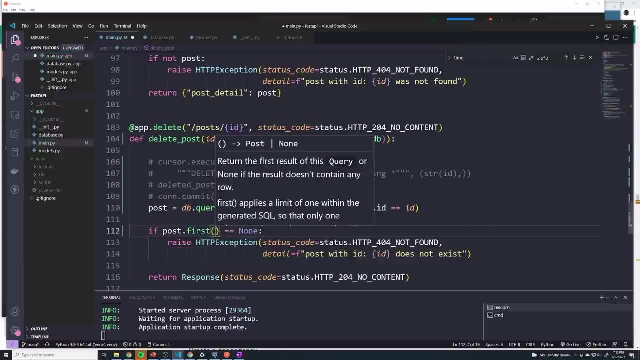 to do is we're going to say: if post dot, how do we actually run this query? Well, we do first, so that's going to query, And so if this returns back nothing, then we're going to raise a 404.. So 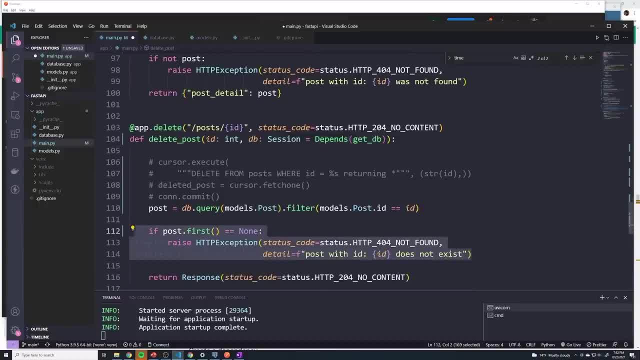 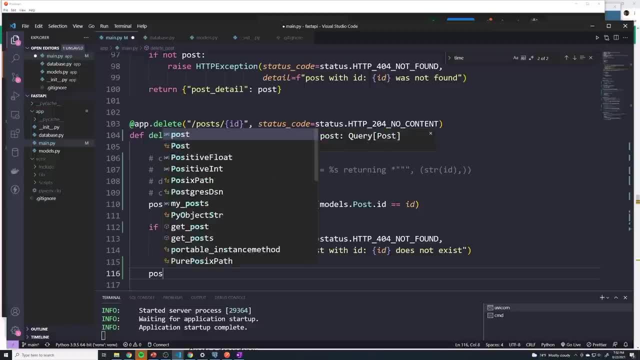 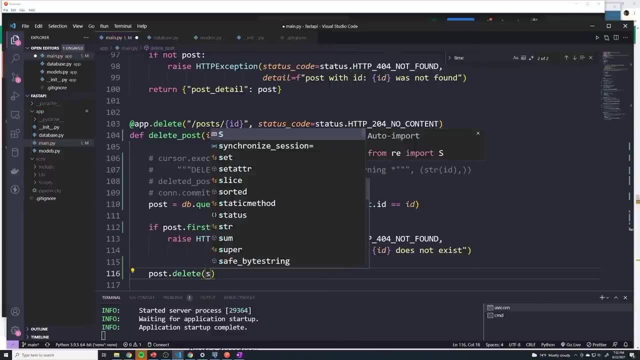 really, we haven't done anything different from what we did here. However, if it does exist, so the outside of this if statement, I'll do a post dot delete And then we'll just say O synchronized session equals false. I believe that's the default. 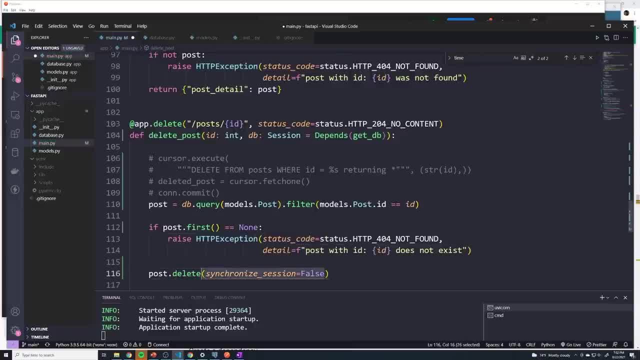 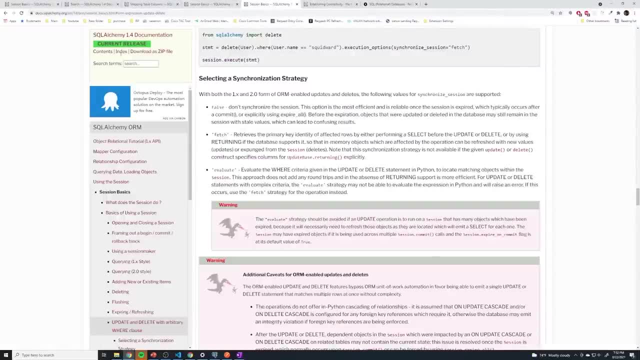 config. Anyways, I don't want to spend too much time going over this. It doesn't really matter too much. But if you want to read about it, just take a look at the document and if you go under, you know session basics- you could see them kind of. 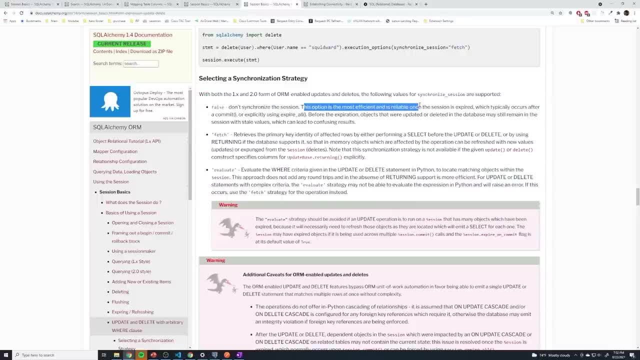 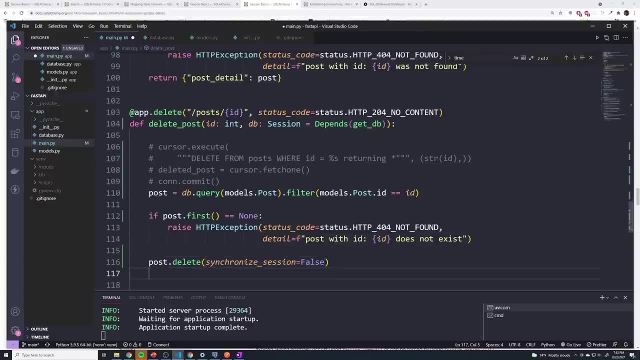 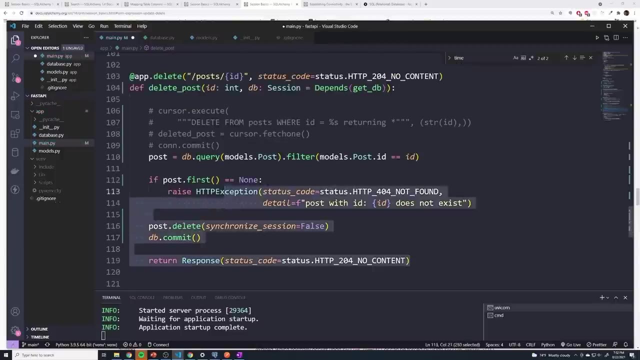 describe all of them, but this option is the most efficient and reliable, so I just went ahead with that one and it seems to work just fine. so this is going to delete the post, but remember, to actually make changes we have to do a DB commit so that'll delete it and then everything else should, and. 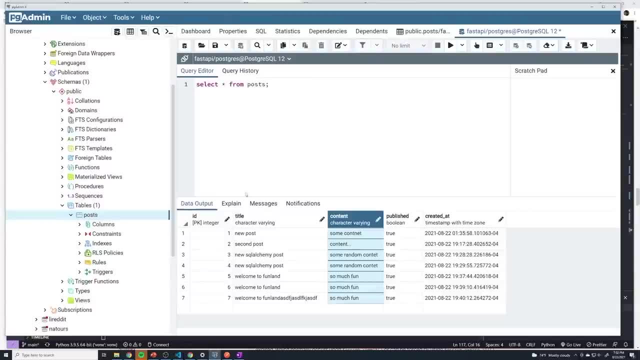 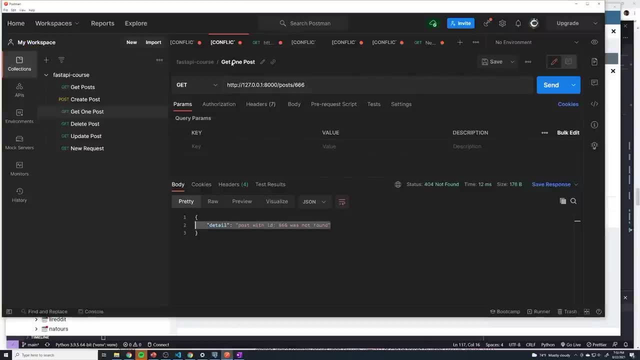 can remain the same. I'm going to go back to my postgres database. we're going to delete post with the ID of six, so we'll go to our. I was postman. we'll go to our delete operation and then we'll do a an ID of. 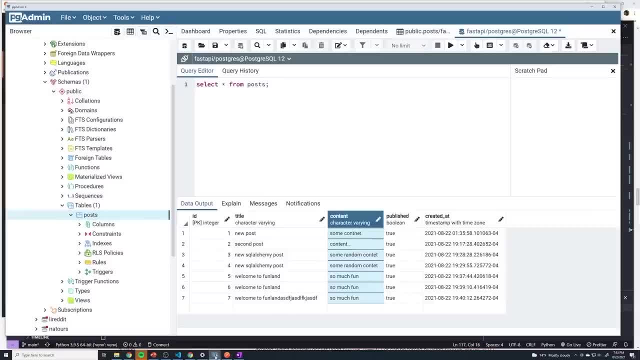 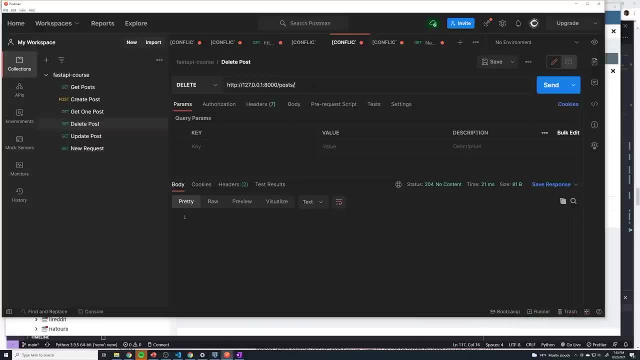 six. all right, seems to work, but let's double check with postgres right now. now we can see that there's no longer a post with an ID of six, and then let's test this out with a random post number that doesn't exist. we should get a 404. 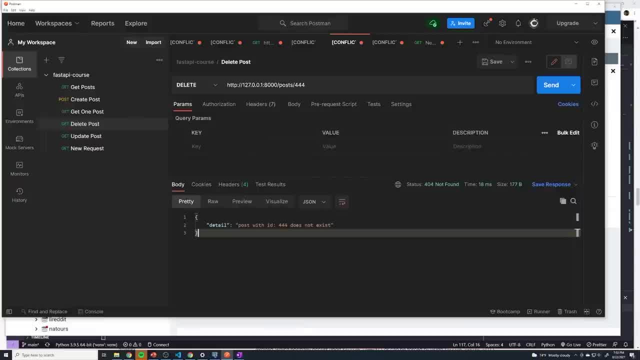 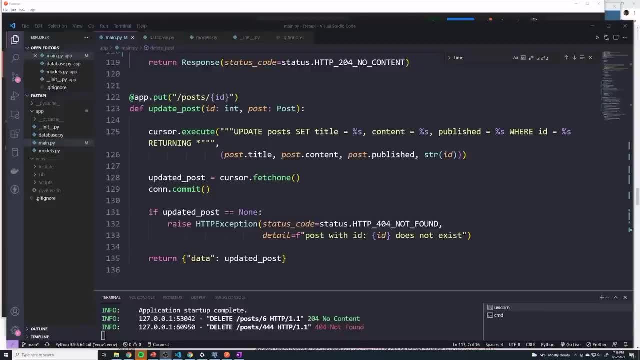 perfect, you okay. so it's time to tackle our final path operation, which is for updating posts. this is one's going to be fairly similar to, you know, deleting a post or even getting a post by a single ID. so, first of all, comment out the previous postgres code and, because we're going to be interacting with the database, let's 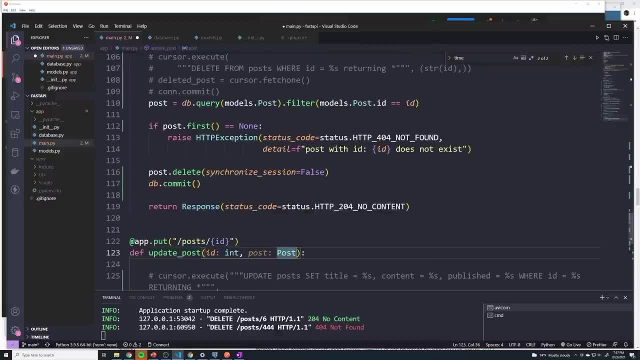 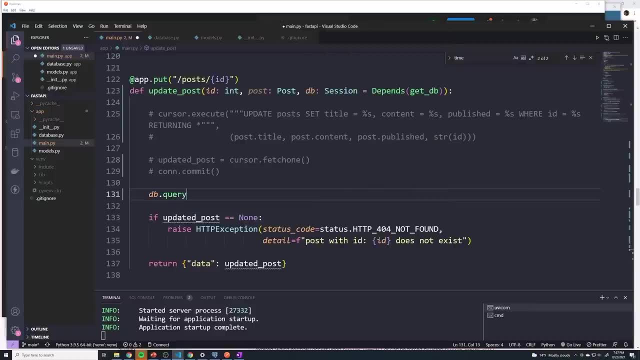 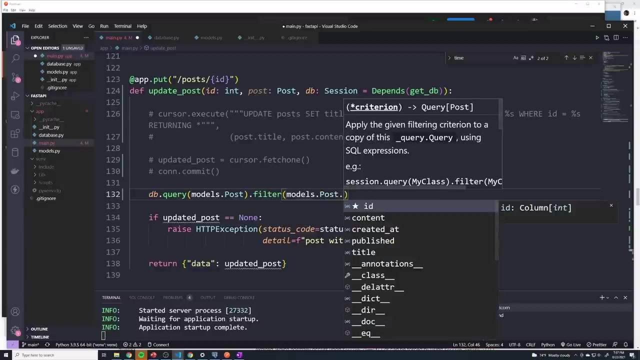 make sure we copy the dependency in this case. and then what we're going to do is we're gonna do the same thing, we're gonna say DB query and query models named post, and then we're gonna filter on the same thing, will say filter models dot post. 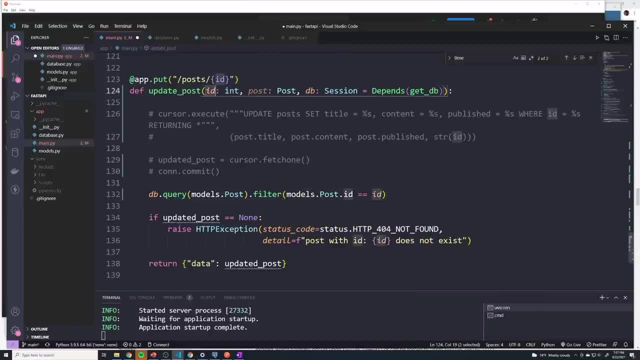 ID and if that equals to the ID that we're passing here, then we're going to find the specific post were interested in. so I'll say I'm gonna save this as post underscore query. so right now I will not actually running the query. were just saving the query because I haven't run it yet, but we'll save it. so we're just saving a new book surhandler a query. we're just saving the query because we haven't run it yet. so this: Make sure to go ahead and click on the termoid to do this in three minutes. and then I'm going to go to one big- I just think we've already got this in here- which is this: Think Come toち is called the TwitterЫModelZaWtestWρι. 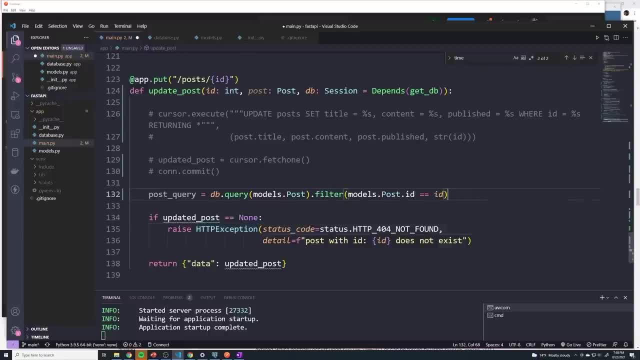 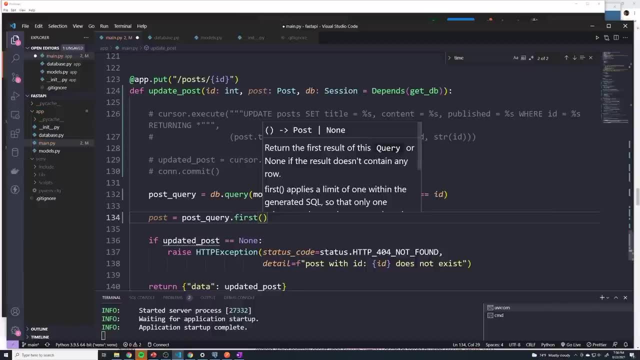 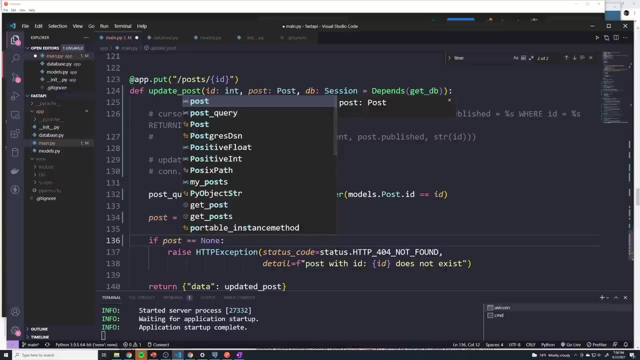 because I haven't run dot first or dot all And we'll say: the actual post equals post. underscore query: dot first. This is going to grab the post if it exists. If it doesn't exist, so say if post does not equal none, or if post equals equals none, then we're. 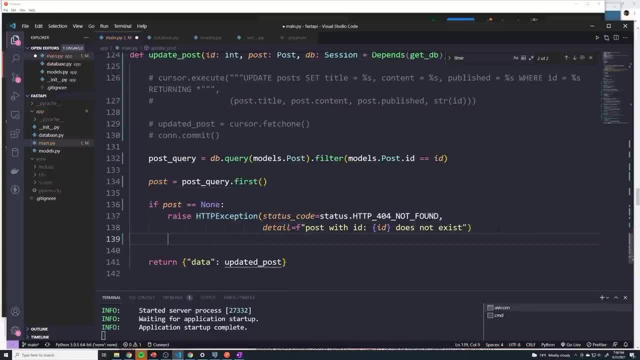 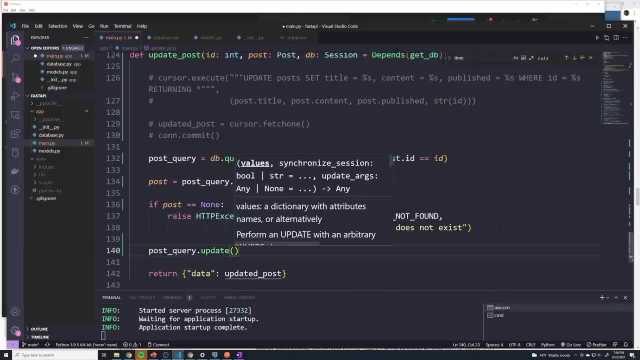 going to send a 404.. However, if it does exist, then we'll we'll grab the query again, say post query dot update, So we can chain an update method. So we're basically taking this query right here And then we're chaining the update method, which would be the equivalent. 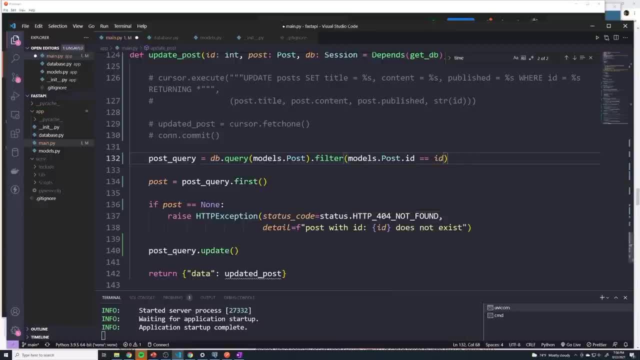 of doing an update right here. Let's say dot update, And then what we want to do is we want to pass in the the fields that we want to update as a dictionary. So in this case, what I'm going to do is I'm 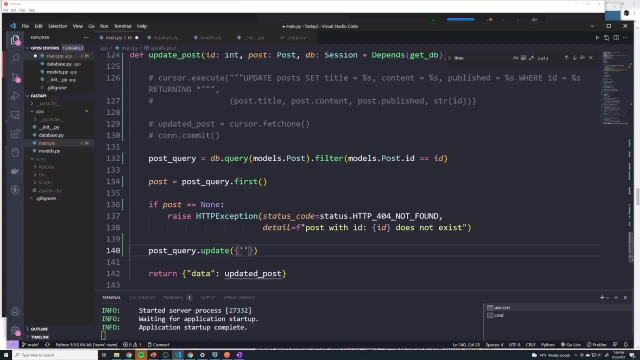 going to hard code the values and just to show you what that looks like. So we'll say title is going to be set to: Okay, hey, this is my updated title, And then the next one is going to be the content we can. 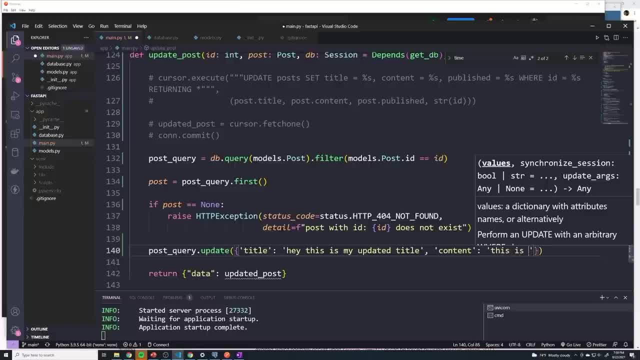 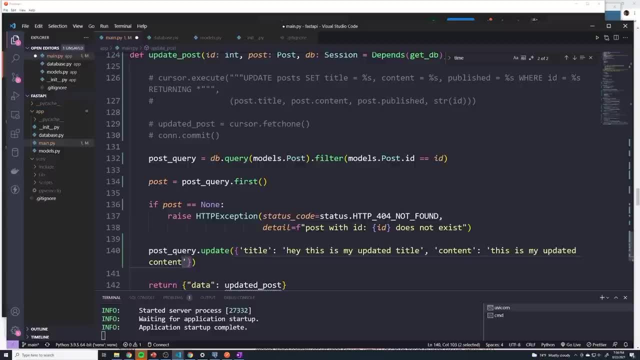 update that to be whatever we want And I'll say this is my updated content. Then we're going to do that same synchronized session equals false as the second property into the updated method. What a synchronized session equals false. And that should handle the update. And then 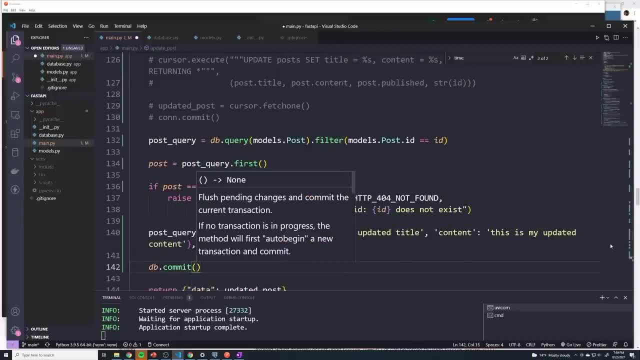 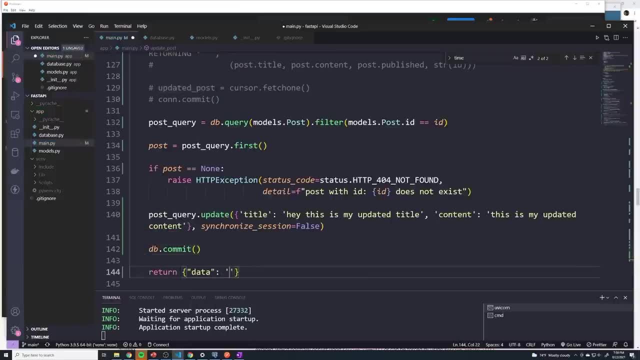 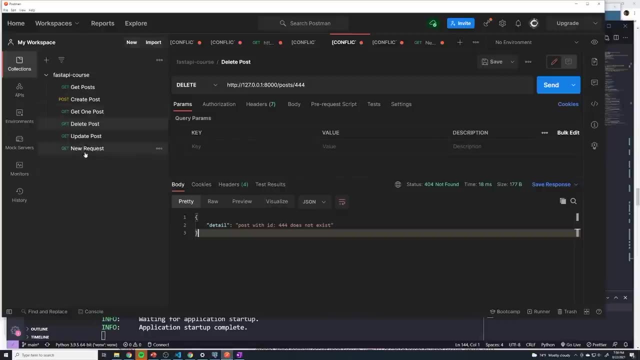 we would just want to do a DB dot commit And right now this updated post doesn't exist anymore. So we're just going to return successful or something, doesn't matter. We're going to change this a little bit later on. Alright, so let's go to our update. Where's our update post? It doesn't really matter what data we 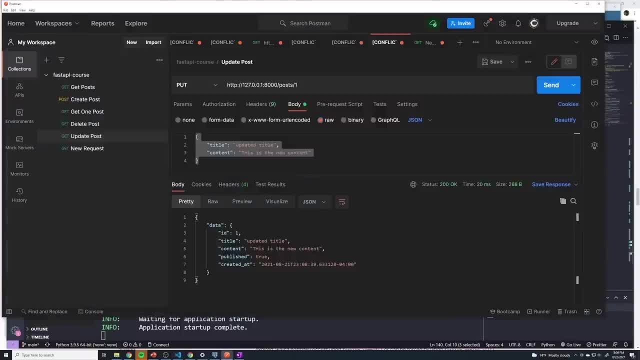 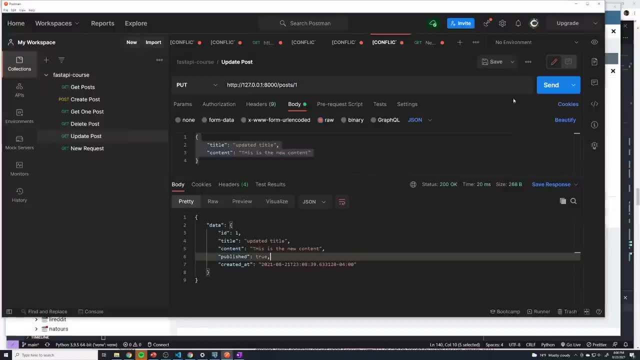 pass in, because we're hard coding the values And so I'm going to update a the post with an ID of one, if it still exists, And it looks like it does. So you can see right now that Now the title is new post. So we'll update this and that's successful, And then let's go to back. 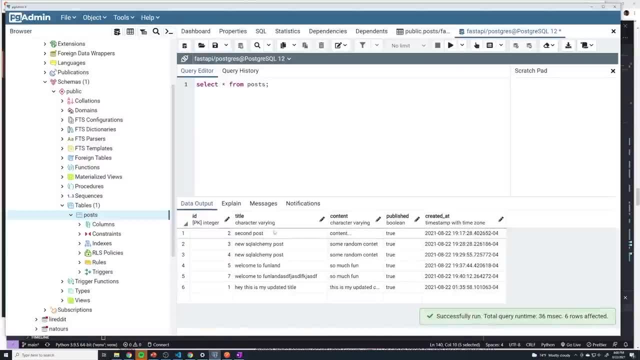 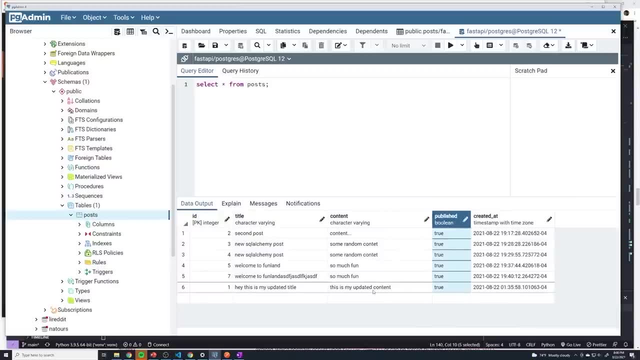 to Postgres, do a query And we can see that. hey look, it got updated. hey, this is my updated title And the content. this is my updated content. So that's all we have to do. we just have to pass. 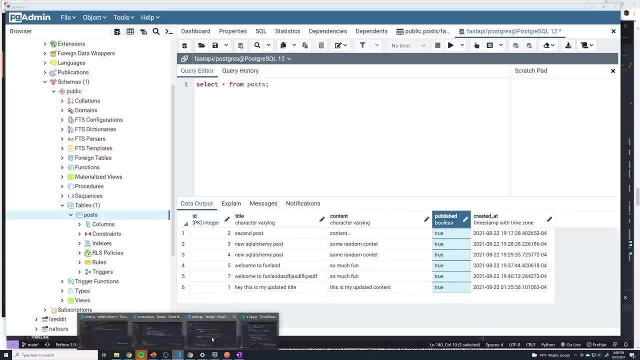 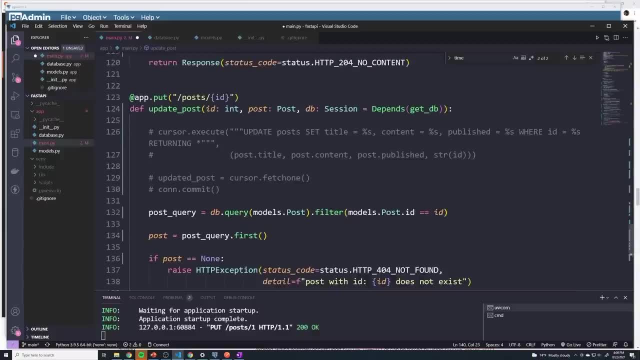 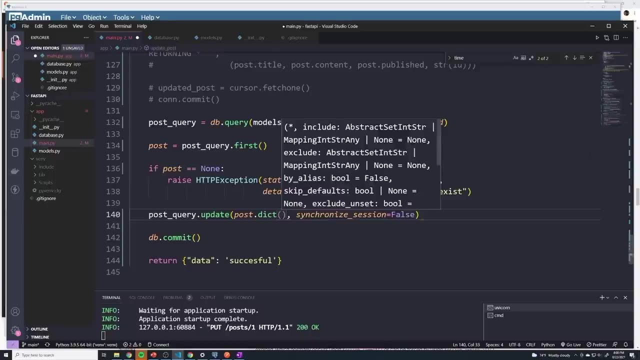 in a Python dictionary with the updated fields. And so instead of passing a Python dictionary, right, we can pass in our post schema, right, So that's going to have all of the updated fields And we can just say post dot dict. that's going to return a Python dictionary. So that should be. 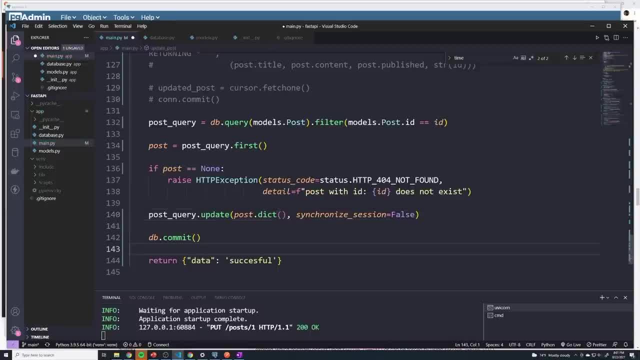 exactly what we're looking for. And then, finally, when it comes to returning data, what we're going to do is we're going to run another query, So we're going to say post underscore query, So we're going to grab this exact query object right here, And then we're just going to get the updated. 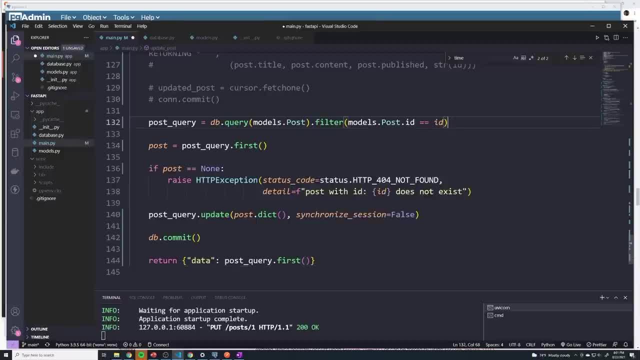 post. So we just grab the first one with that specific ID And then it should return that. So hopefully you guys understand And I'm just going to quickly recap exactly what we did. we set up a query to find the post with a specific 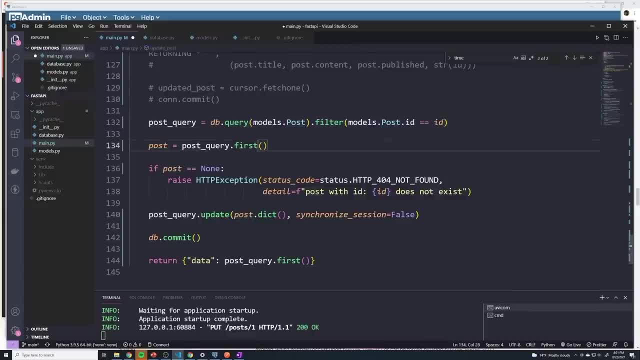 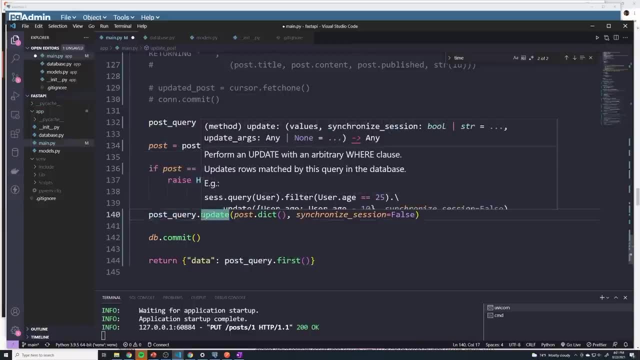 ID, then we're going to actually grab that specific post. So we run that query by grabbing dot first. If it doesn't exist, we're going to run a 404.. But if it does exist, then we can change the update method to the same query object so that we can update it And we pass in the fields that we want. 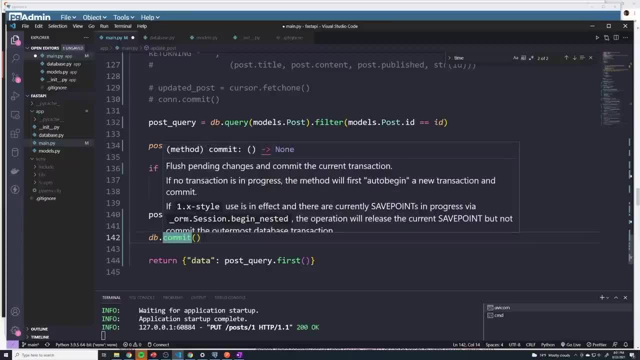 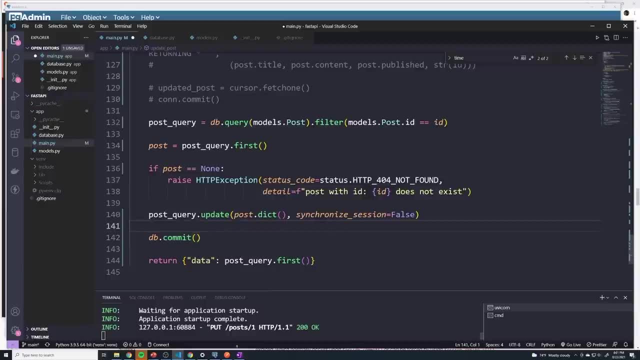 to update, we'll commit it to our database. Then, after all of that's done, we want to make sure we get the updated post and send it back to the user, So we do post underscore query that first. Let's test this out And I'm going to put in values, because these values now matter And 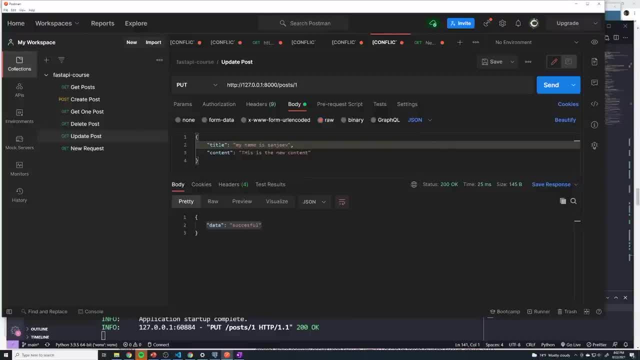 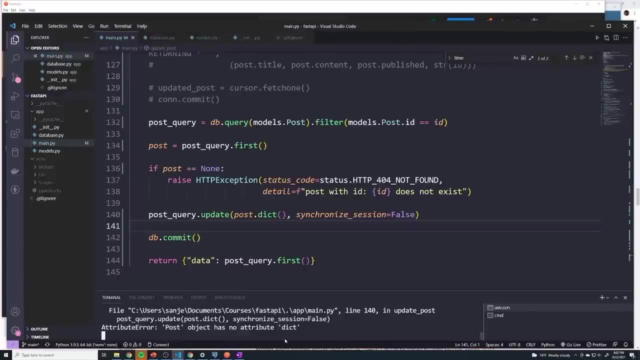 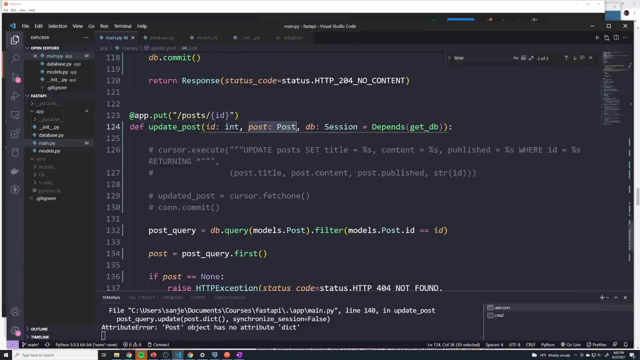 I'll say: My name is Sanjeev, Python is fine, So let's try this. What happened here? Okay, I forgot to save It, send. we get an error And I realized we have a little bit of an issue. So this the schema that we get where we extract: 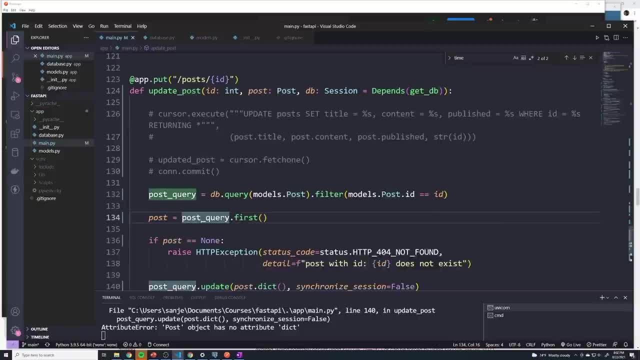 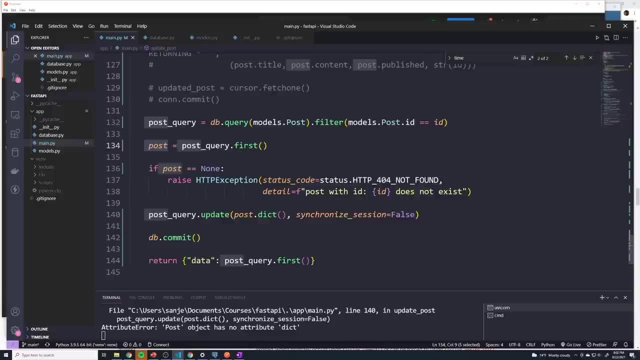 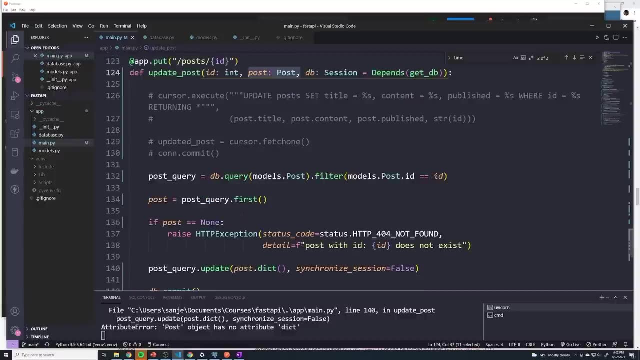 all of the body fields is named post, But then we also save this as post as well, And so this leads to issues because they're both named the same thing, And so I'm trying to- I'm trying to convert this to a dictionary, which only works on the pydentic model. It does not work on our SQL. 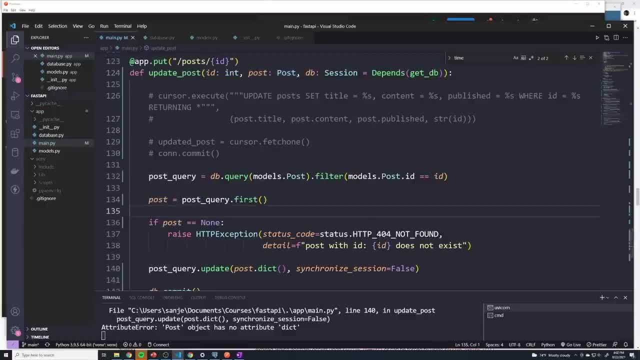 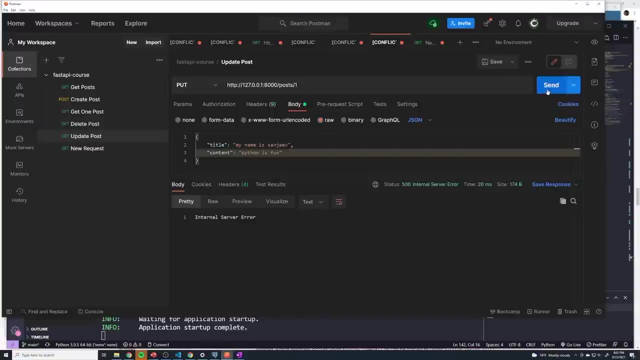 alchemy model, So we're gonna have to rename these. I'm going to name this updated underscore post, And then here this is going to be updated underscore post. Now, let's try that again. seems to work. Let's check our database, though, And we 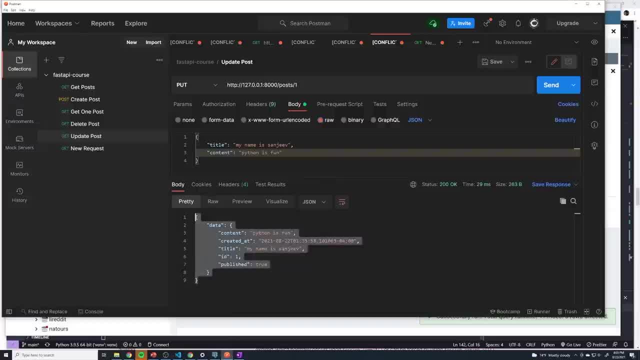 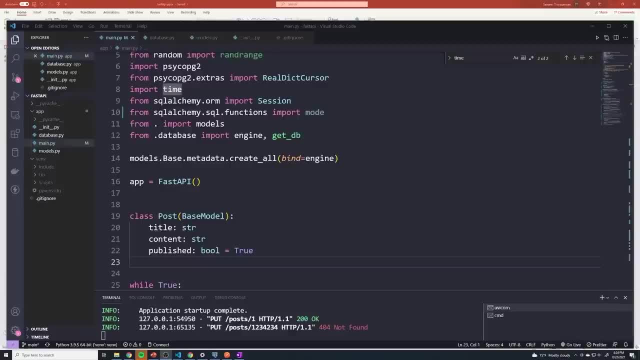 can see that it was successfully updated. And then let's try to update something that doesn't exist And we get a 404.. Perfect. Before we proceed Any further, I do want to provide some clarifications on what are the difference between a schema or 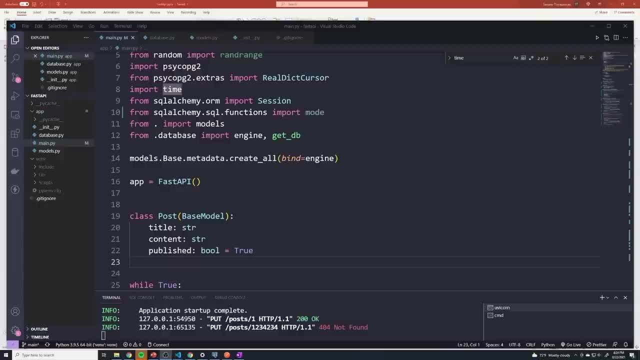 pedantic model and our ORM or SQL Alchemy model, And I think it's important that you guys understand that, and I do realize that there could be potentially some confusion as to what's the difference between them. Ultimately, what are they trying to accomplish And why do we have both of? 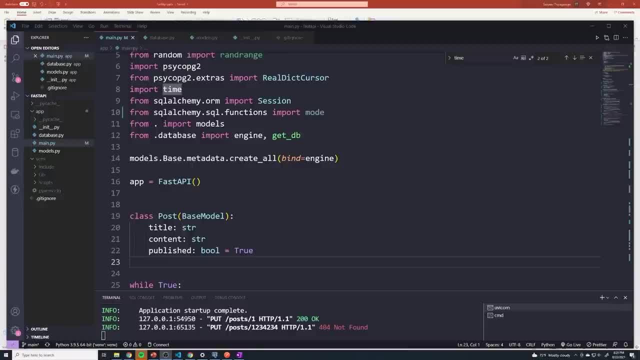 them. so I've created a couple of slides and hopefully that helps sort things out and hope and hopefully it provides a little bit of clarification if you guys were confused at that. But just to to look at our code, you'll notice that in our mainpy file we have one class called post. here 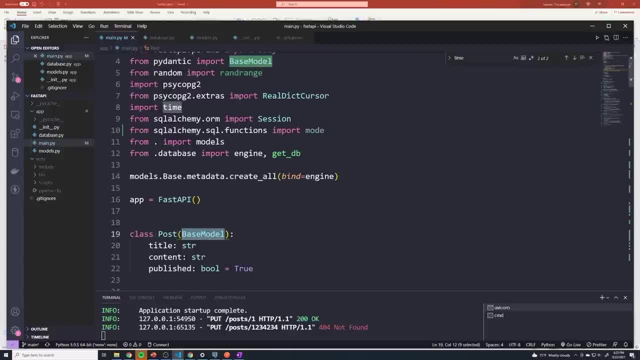 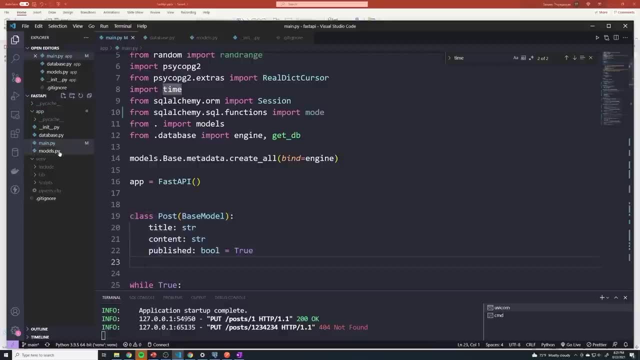 And this is extending base model, which actually comes from the pydantic library And you can see we're importing pydantic right here. So this is what's referred to as our schema And we also have our, and I don't even want to explain it yet. I hopefully you guys already know what it is. But 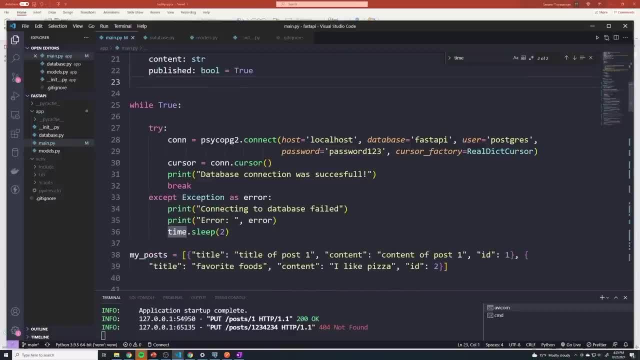 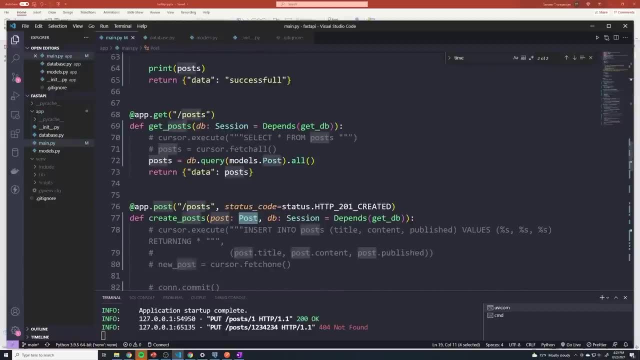 I have a couple of slides that hopefully make it a little bit more clear. But just to kind of show you where this is being referenced, it's being referenced in our path operations, So if you go to, you know our create posts which, wherever that is right here, you can see that we're 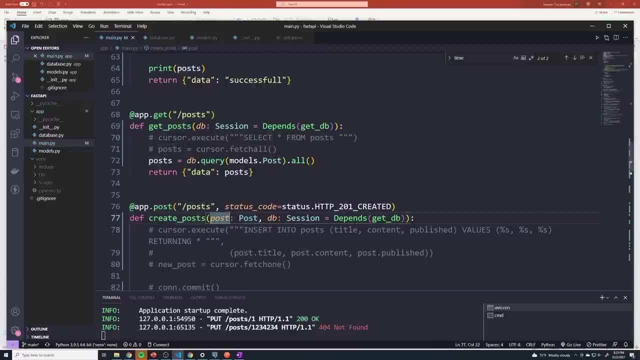 passing that in right here and then saving into a variable called post, So we're referencing it right here. This is all about defining the shape of a request, And so that's the pydantic model. The other model is the one that we have in modelspy, which is the SQL alchemy model. So this: 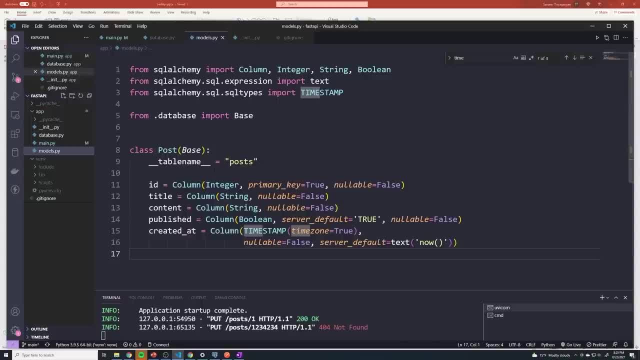 SQL alchemy model defines what our database, our specific table, looks like. But let me pull up the slides just to show you guys, you know, with some nice diagrams. So hopefully you guys get a better idea of what that looks like And then we'll see you in the next video. 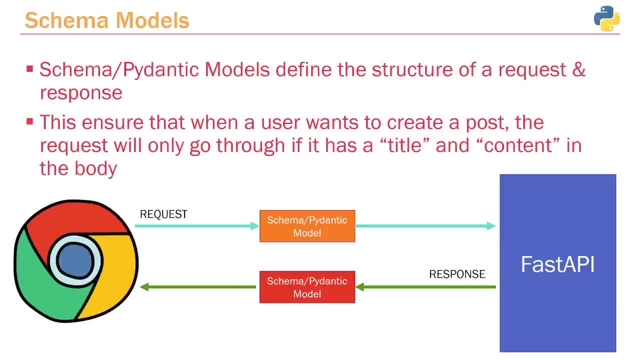 idea of what that is. All right, so let's start off by going over the schema models or the pydantic model. So the schema or the pydantic model defines the structure of a request and a response, And so that way you know, when it comes to creating a post, we can define exactly what the 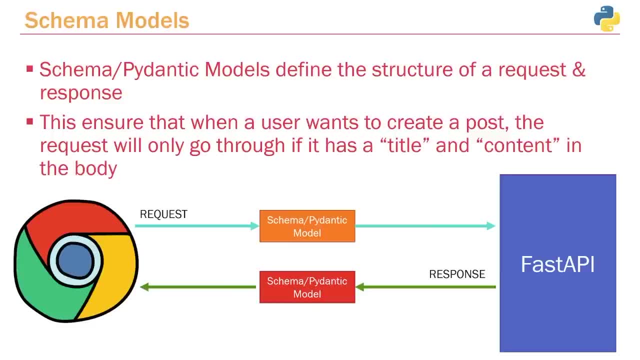 request should look like. So when we create a brand new post, we need their user to provide what's the title of the post, what's the content of the post, And optionally they can also provide if it's published or not. but we've provided a default value So they don't actually have to. 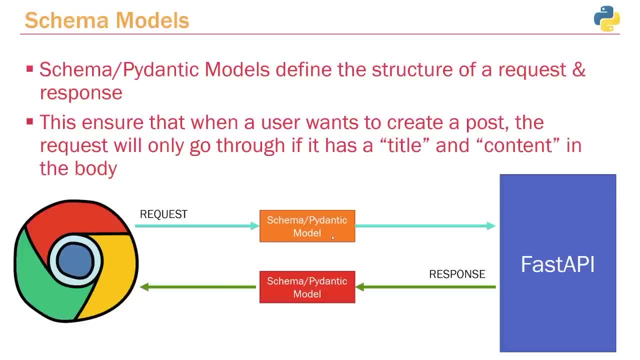 send that. So what we do is we take the request and we're going to send it to the user, And so we pass it through the pydantic model. the pydantic model will perform a little bit of validation to make sure that all the fields that we need to actually create a brand new post are. 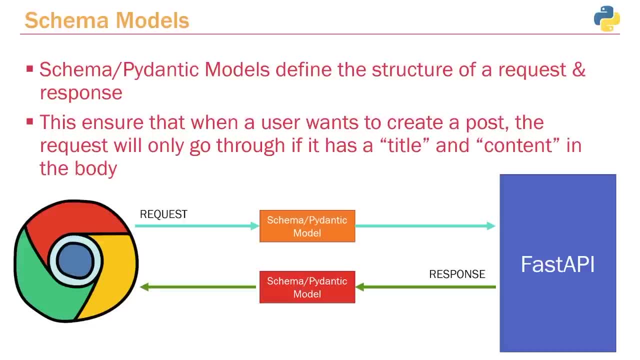 there and that they are of the proper type. So if it's a title, it shouldn't be an integer, And if it's the published property, it shouldn't be a string or anything. It's just a simple Boolean. So that's what the pydantic model or the schema model does. It's just there to provide some 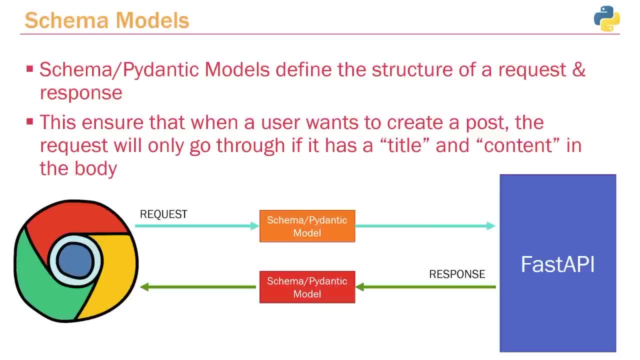 validation to ensure that the body, all the data fields provided in the body of a request, match up to what we want. And that's important because we don't ever want to give the clients- which is the web browser or the mobile phones or anything like that- freedom to do whatever they want. we want to tell them 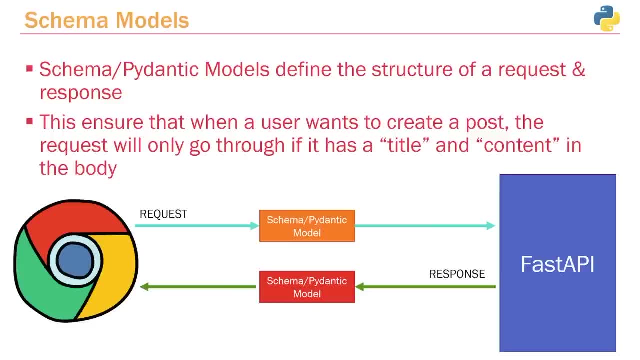 exactly what we need for each specific path or route, And that's for the request. However, we can also do this for the response, And we haven't actually done that yet, But we can actually define exactly what that response should look like. So you know, as our, as our models get more complex, 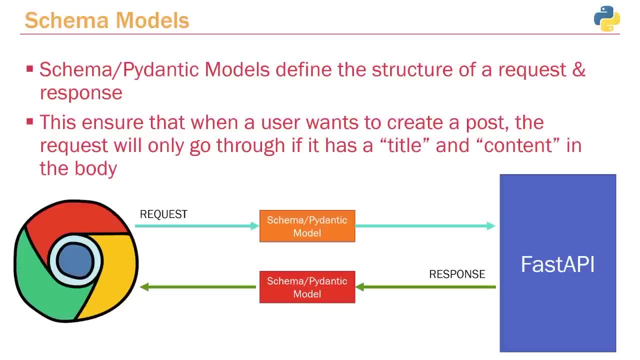 as our database gets more complex, there's gonna be a lot of fields, when it comes to your posts and your users that you may not want to send back to the client when we send a response. So we can actually define a model to dictate fast API. 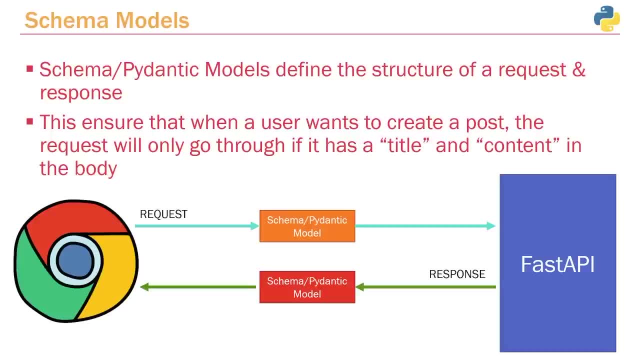 exactly the data fields that we should be sending back, And so that's what your schema and your pydantic models do: they just ensure that the request and response are shaped in a specific way. Now, the other model is the SQL alchemy model, So this is the one that we've been working on with. 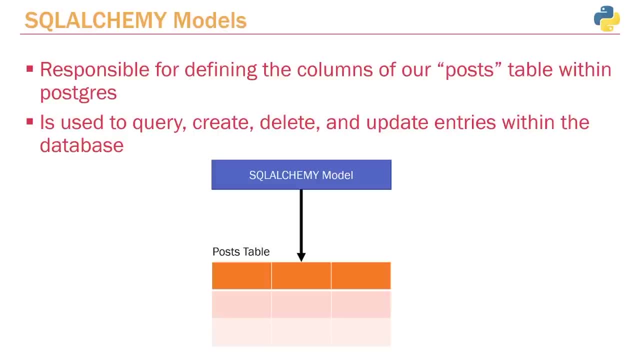 the past couple of lectures And these are responsible for defining the columns of our posts table within Postgres Right. so it's going to define all the different attributes within a specific table and then we use that post model to perform queries to our database. we use it to 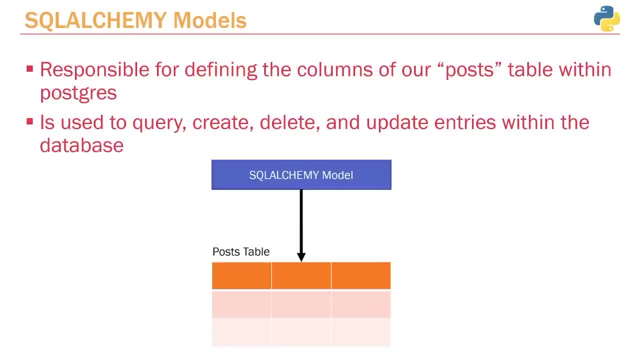 create, delete and update entries within our database. But this model is fundamentally different than the pydantic model, So that's why I created this video. I just wanted to make sure that you guys understood what were the differences between those and understand why we need them both. 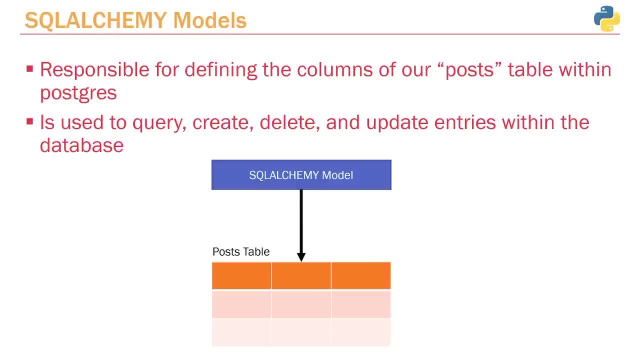 Technically we don't need the pydantic models, But you know, when it comes to building out API's, you want to be as strict as possible when it comes to what kind of data can we receive and send to the user. 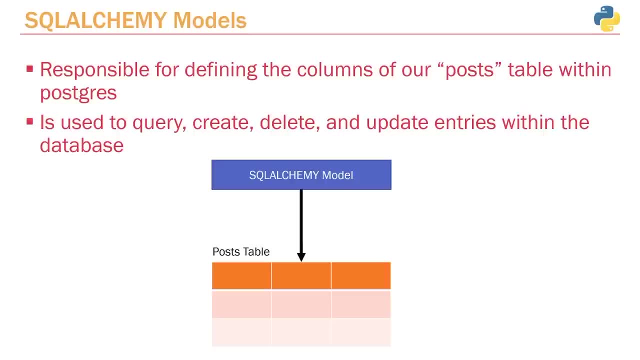 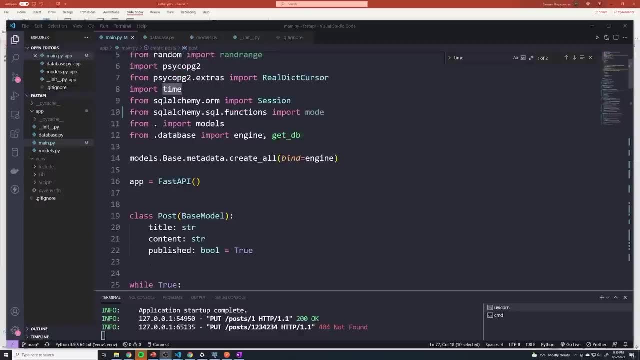 And so pydantic just ensures that, you know, everything just matches up with what we expect. So in the last video I described the difference between a PyTantic model and a ORM model, And there's a couple of things I actually want to do with our PyTantic model. So we've just got one right here where. 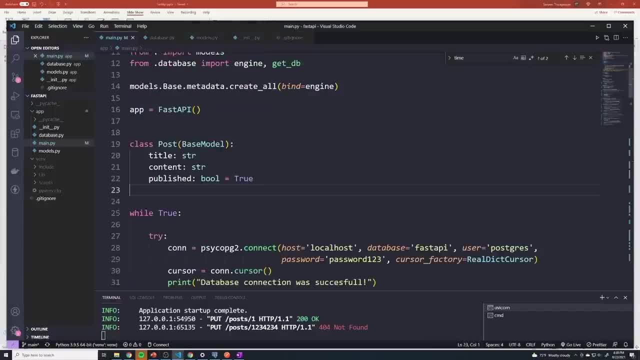 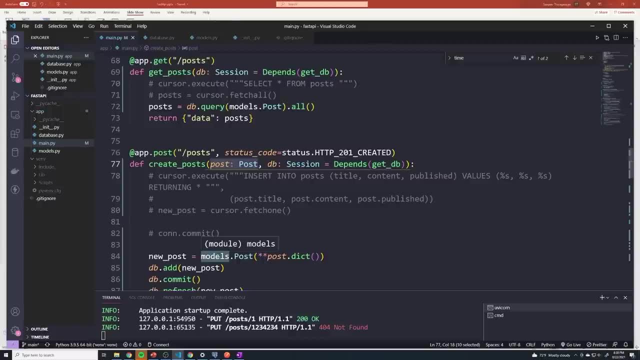 we define what a request, what a post should look like, And we use that in a couple of places. So if we go down to create posts, we can see we use it there. So it's going to define the structure of the data that we receive from the front end when we want to create a post, And I think we 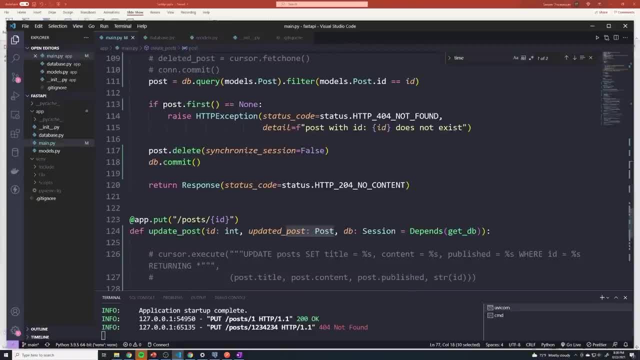 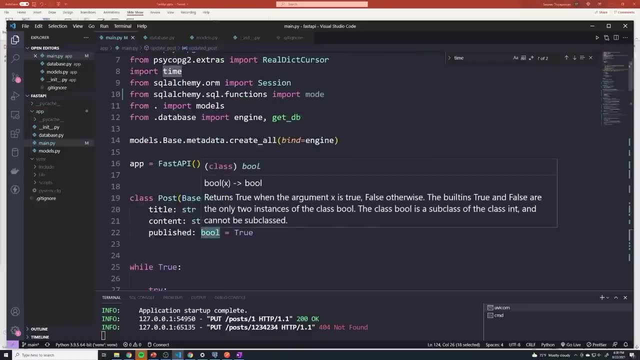 also provide it for maybe updating a post. Yep, we also use it for updating a post as well. So what I'm going to do is I want to create the schemas or I want to move the schema. in this case- remember, this is what's referred to as a schema- I want to move that to its own file. 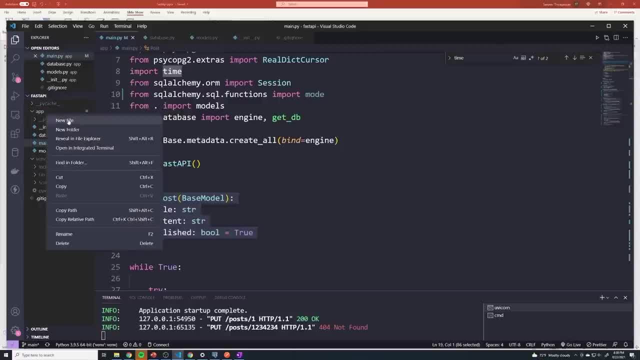 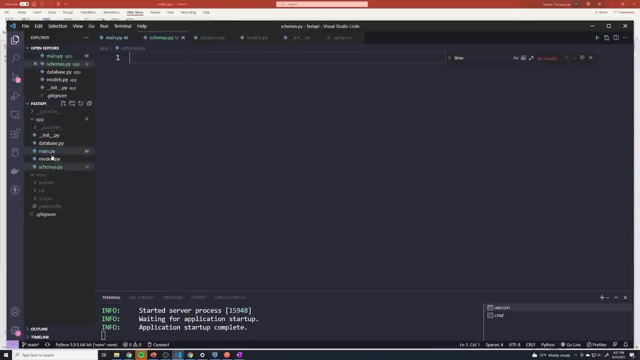 just so that we don't clutter up our mainpy file. So I'm going to go under app, I'm going to do new file And I'm going to call this schemaspy, And then, within schemas, if I go to my mainpy file, 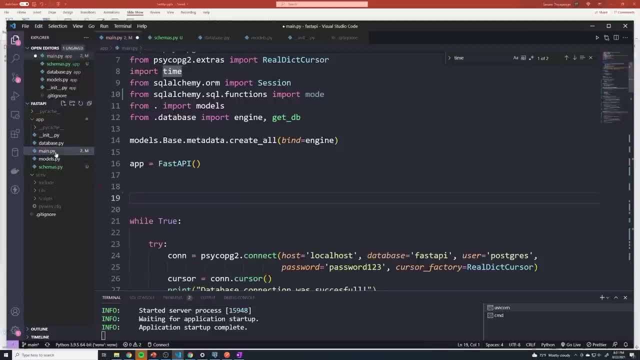 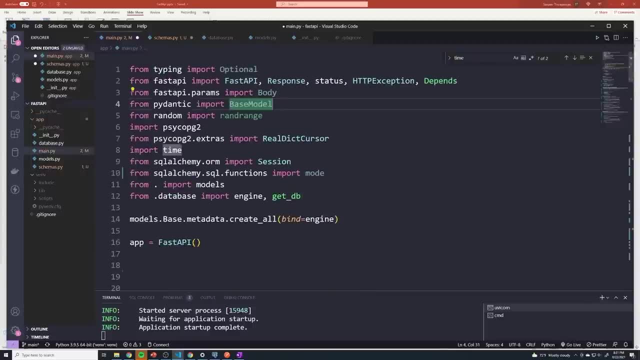 I'm just going to cut this out And we can paste it in here, And there's going to be a couple of things that we have to import And so if we go to our mainpy, we definitely need pydantic. That's really all we need. 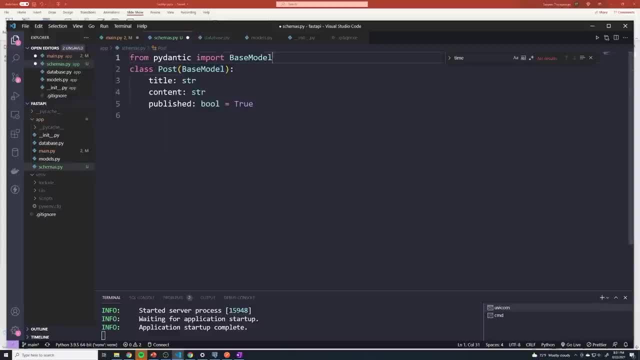 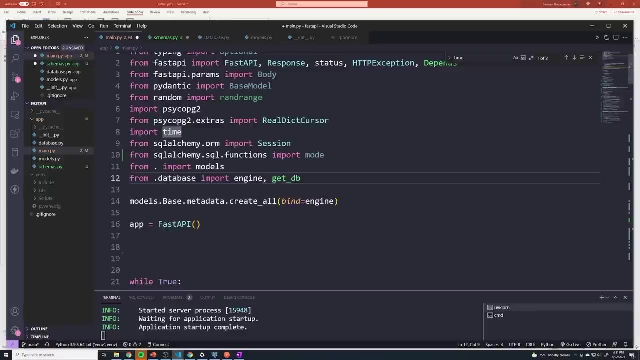 actually. So if I go there and then paste that into there, we should have no issues. And then you know this is going to actually break our application because we need to actually import this specific schema. So if I go into mainpy we can see here I'm doing from dot import models. So 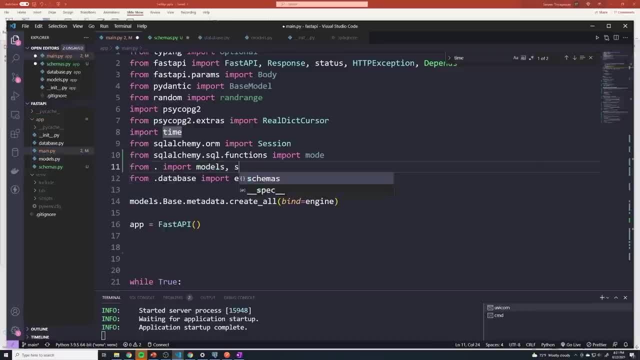 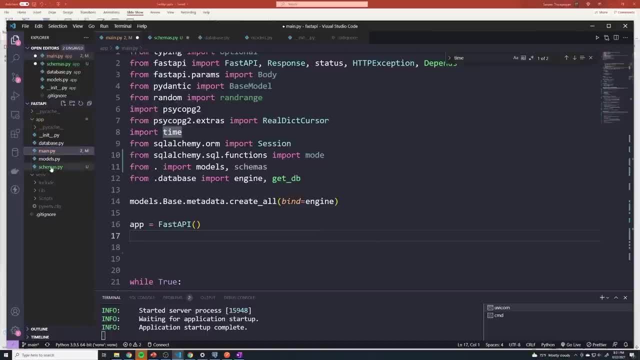 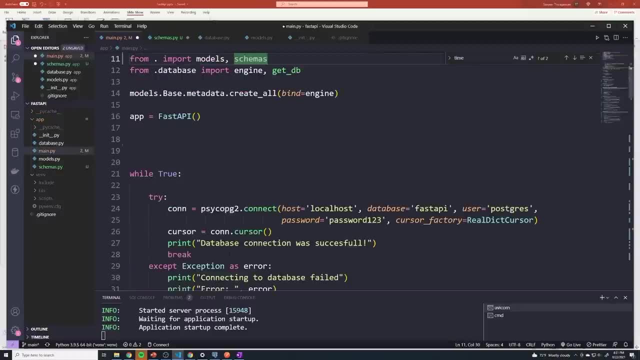 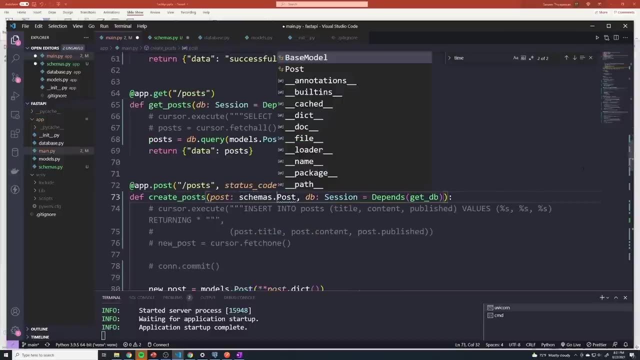 schemas as well. And so now to actually access this specific class post we just have to go in our mainpy file and the reference schemas dot post, And so anywhere we use post- which should be right here- we can do schemas dot post. And then in our update post as well, we can do the. 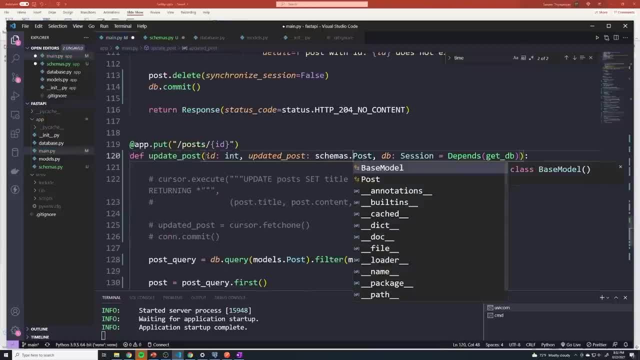 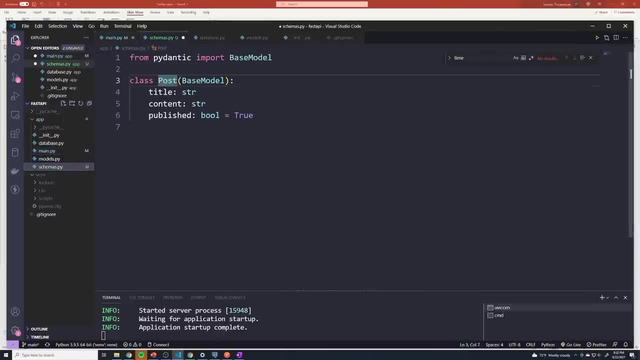 same thing is going to be schemas that post, because now we're importing it from another file And what I'm actually going to do is we're going to restructure this a little bit. So what I'm going to do is remember these are regular Python classes And so we get all of the abilities that 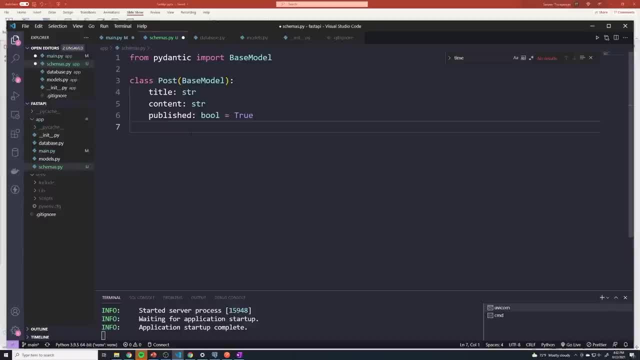 we have when it comes to inheritance, when you come, when it comes to working with these classes. So what I'm going to do is we could define a couple things right. we could have one for, we could create a class for create post. actually, that should be capitalized. So create post. 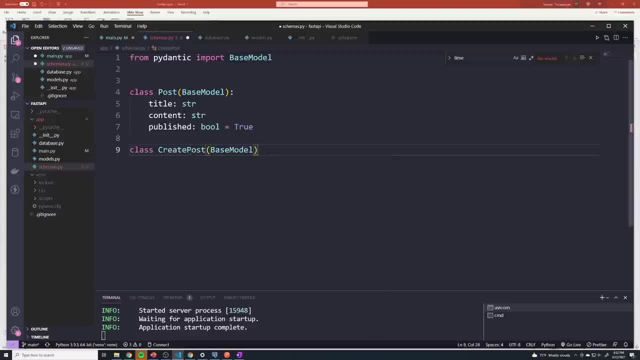 And that's going to extend base model, And then we're going to import the schema, And then we're going to import the schema, And then this is going to have all the fields that we need from the user when it comes to creating a post, And so that's what this would be in this case. 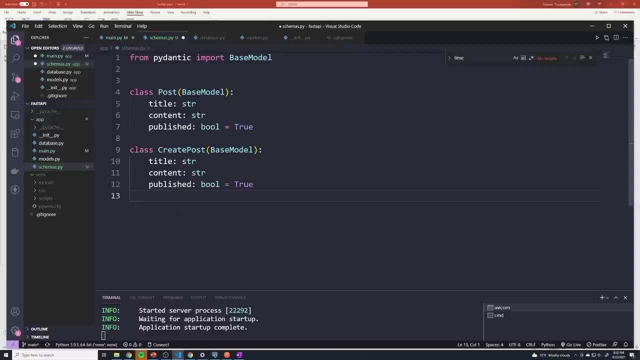 And then remember we also need to handle updating posts, And so we could create another model for that. So in this case I could call it update post And once again, that's going to extend base model. And when it comes to the fields that, 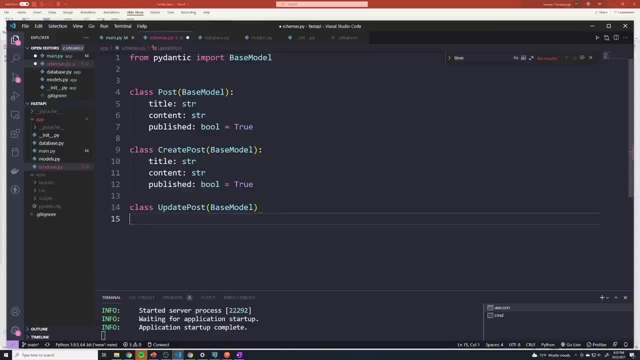 we use for an update post. it would be the same exact thing, right? Whoops, that should be right here, And I don't know why it's doing that. And so at this point, right, we could then have two different classes for each specific. 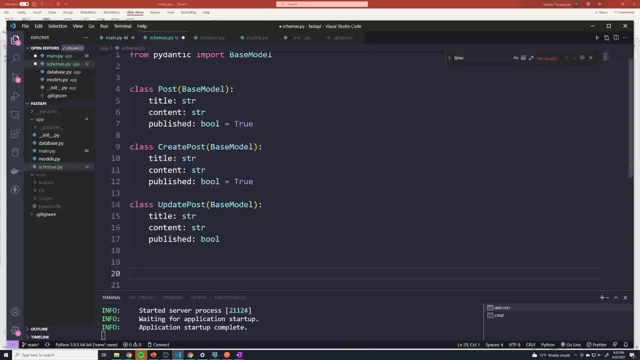 specific request, And that's a perfectly valid use case, because, when it comes to creating, they should provide a certain amount of fields And then updating it might be completely different, right? Because you know, let's say, in our application we wanted to make it so that the 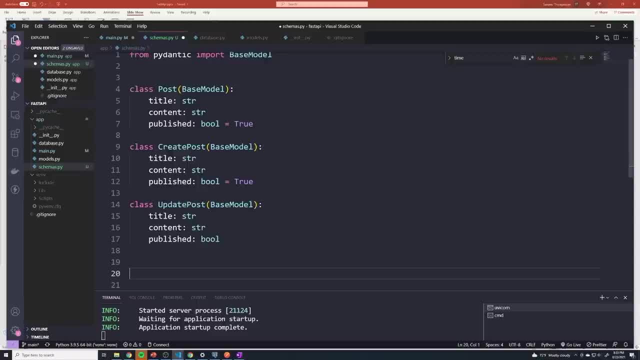 user can't ever update a post. they can only update one property And that's the publish. So they can just change whether it's published or not. we could remove this And this is going to make it so that the user isn't allowed to provide any other fields. they can only. 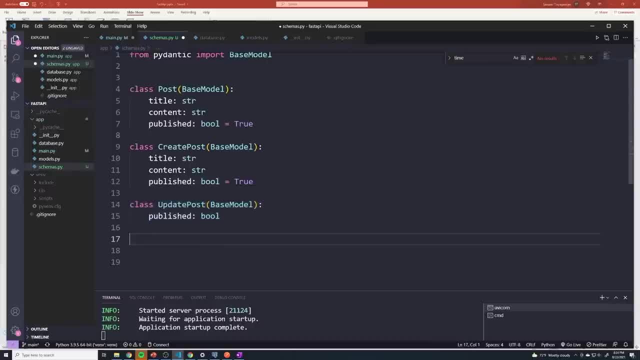 pass the published field. So that's why we would want to create different models for each of the different requests. But what I like to do is, instead of having one for create post, one for update post and then one for the, you know, we have to eventually create models for the response. 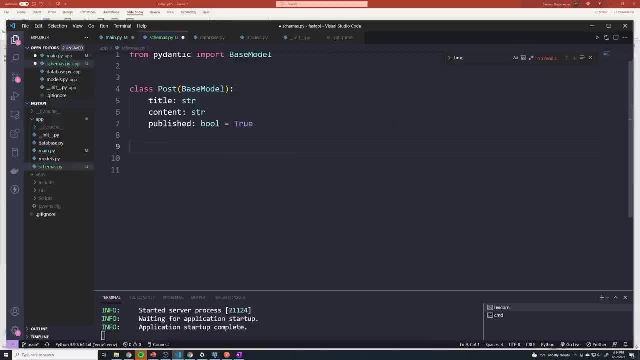 what we're going to do is we're actually going to delete all of this And we're going to create a class called post base. So I'll do class post base and then base model, And so this is a regular class. we can just copy all of these fields. 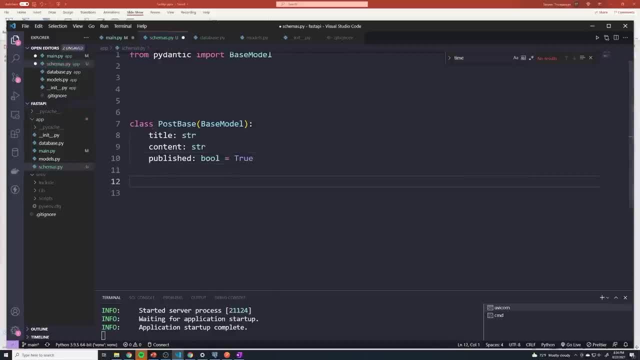 And then we can extend that class. So I can take this post base class And I can extend it and say class: post create. I want to extend post base, we can say post base, And so it's going to by default. 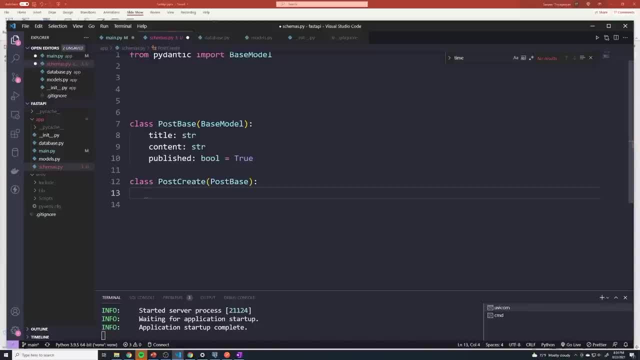 automatically inherit all of these fields, And so we can just say: for creating. we could just say pass, which means it's just going to accept whatever post bases. So post create is essentially the same thing as post base, But then we can create a brand new one called class. I don't know. 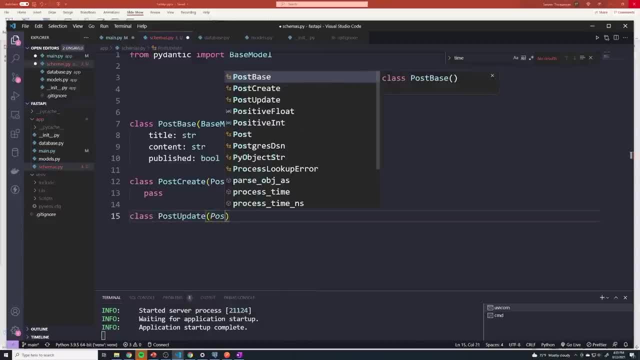 post update And that's going to extend post base And we can say that for updating we can pass in whatever specific fields we want to add in as well. So that gives us flexibility because we can make use of inheritance. So for now I'm going to remove post update and we're just going to keep. 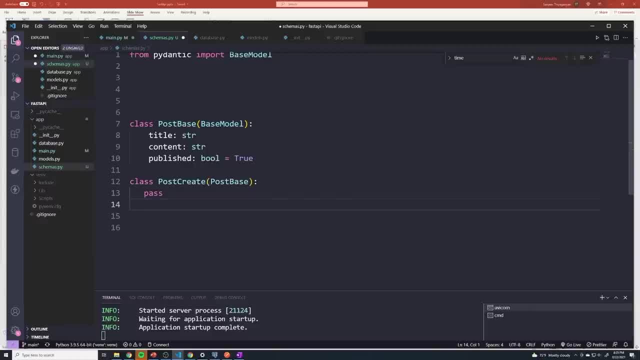 it as post create, Because you know, updating and creating is going to be fundamentally the same And that way we can just kind of piggyback off of this post base model and then just create brand new models based off of this. So what I'm? 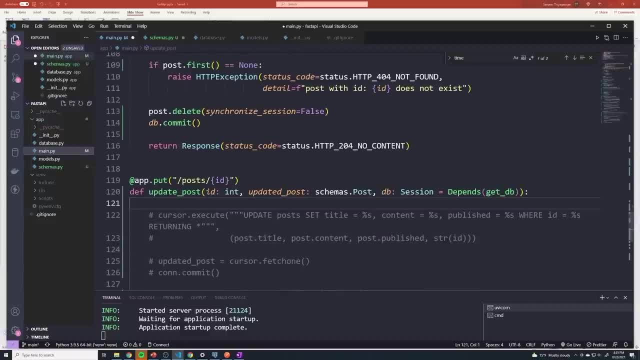 going to do is go into my mainpy file And then, for schemas, actually let me save this. Then my mainpy file. there's no longer a post. it's going to be post. actually, it's going to be create post. 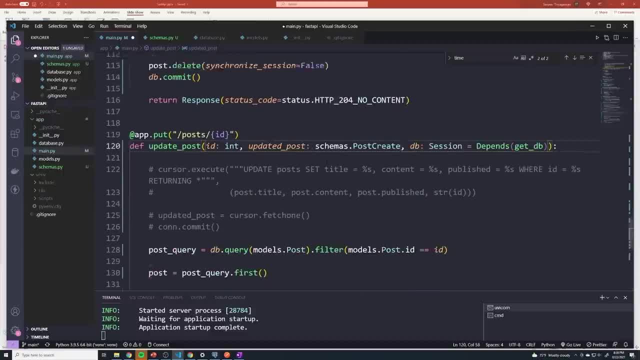 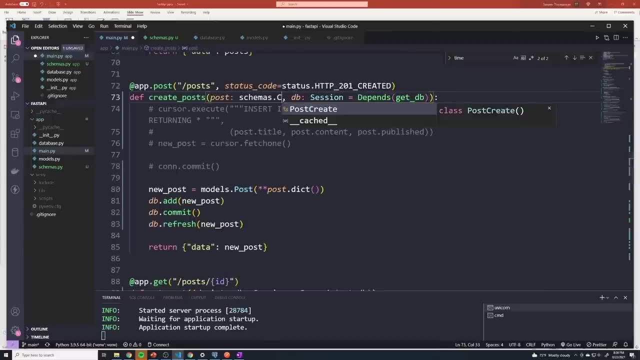 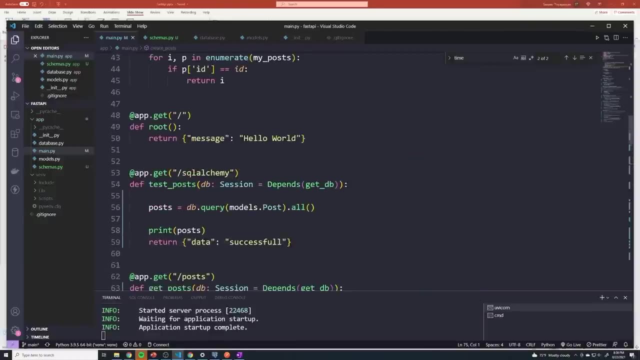 create. I'm gonna do the same thing for update as well. That was the update, Actually. so then the other one is for create post, And then this is going to be schemas dot, post, create. Alright, and the last thing that I want to do in this video is we're going to just delete this test route that we had. 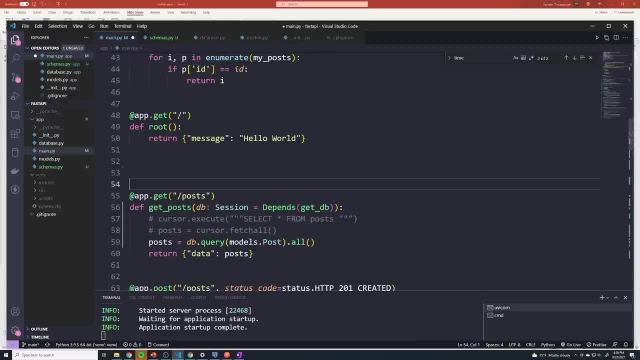 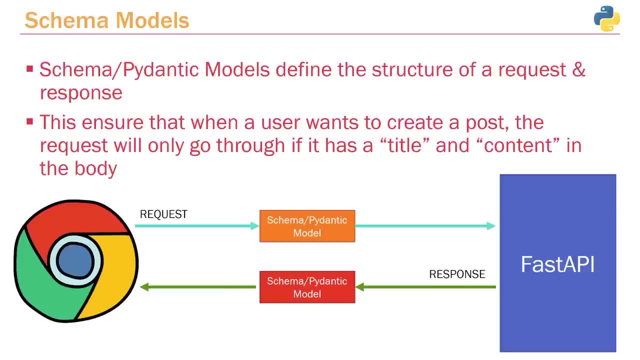 defined when we were learning about SQL alchemy. We don't really need that anymore. And then, in the next video, what we're going to do is we're going to tackle sending a response back Right And, as I mentioned, within the slide deck. 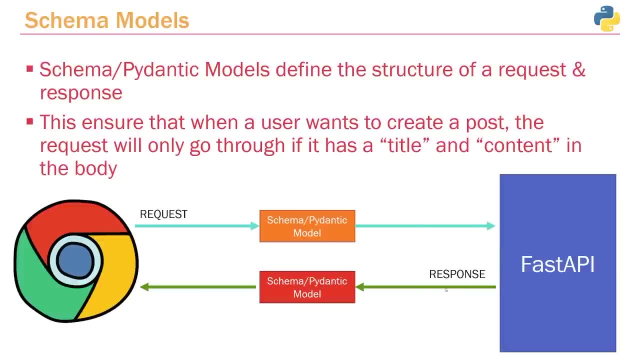 just like we can define what a request should look like, we can also define exactly what a response should look like. So we're going to do the same thing. we're going to define a pydentic model for a response, for what a post should look like when we send it back to the user, so that it sticks to a very specific schema, and then we 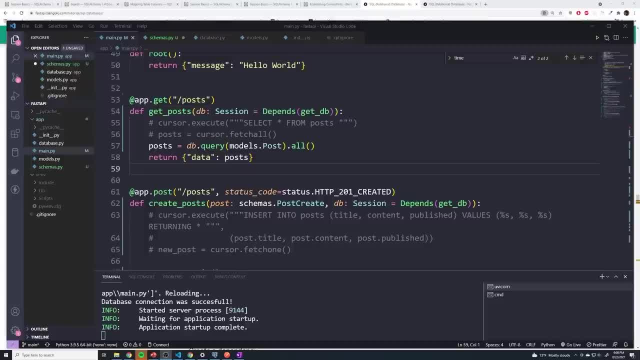 don't end up sending data that we don't actually need to send to the user. In this lecture, we'll take a look at how we can define a pydentic or schema model to define the exact shape of a response, Because right now, if you 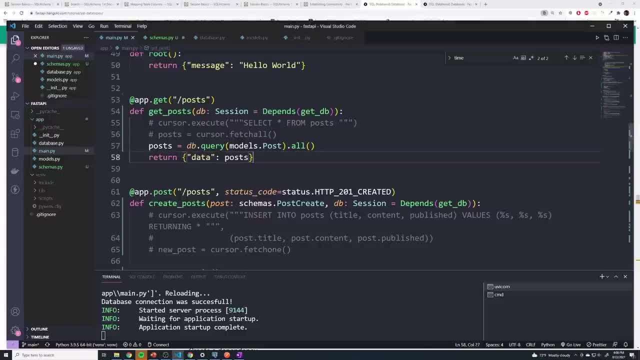 actually see any of our path operations. what we do is we just return a post or multiple posts or an updated post, And whatever data we get back from the post, we just send it back to the user. And there may be times where maybe you don't want all of the 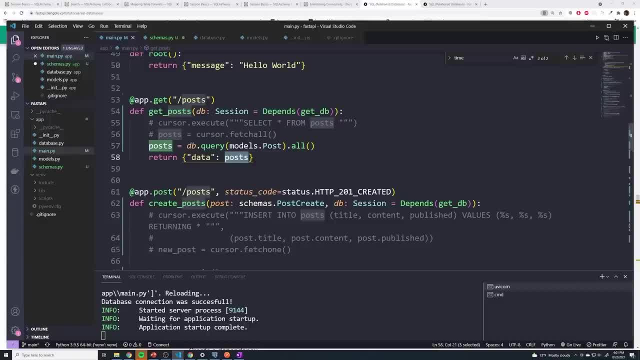 properties or all of the attributes and columns from our POST table to get sent back to the user, because you know potentially that could be sending him back information he shouldn't know about, Especially when it comes to you know, like your your user account right when a user logs in, we 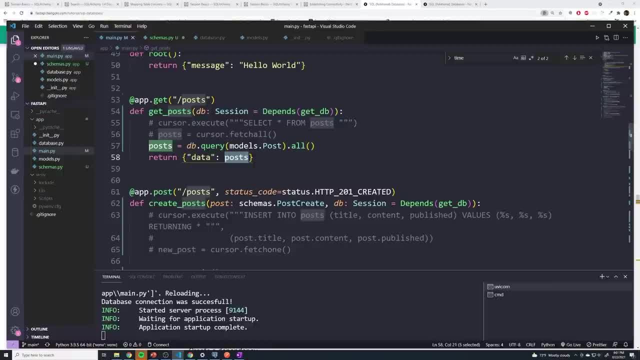 don't want to send him back his password. he already knows his password. We don't want to continuously transmit information like that. So there can be times where you do want to remove certain fields or properties, And before we actually get to performing that, we're going to do a little. 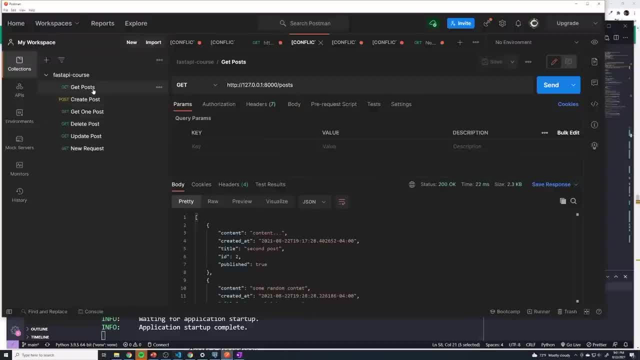 bit of cleanup, Because if we go to really any one of our requests, like if I go to get posts and hit send, you see that we have, you know, within data. we then have the list or array of all of our posts And if we look at create posts, right, you can see we always have data and then 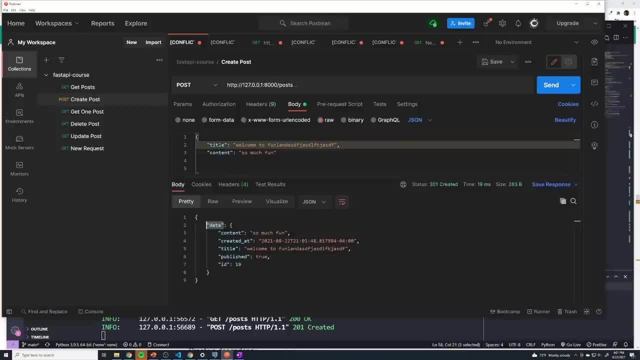 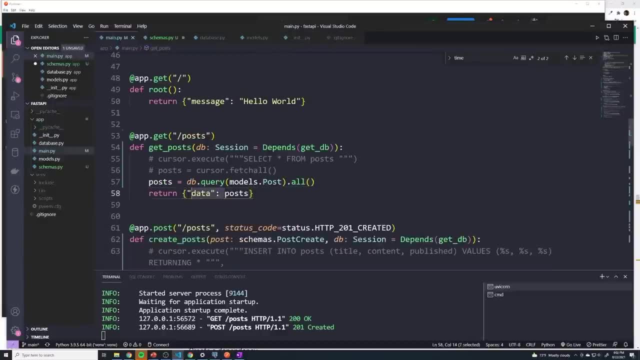 the actual post. I'm going to get rid of the data field just because I think it's unnecessary And it kind of clutters things. So what we'll do is, within all of our path operations, we're going to just remove data And instead of returning- you know a dictionary, we're just going to return. 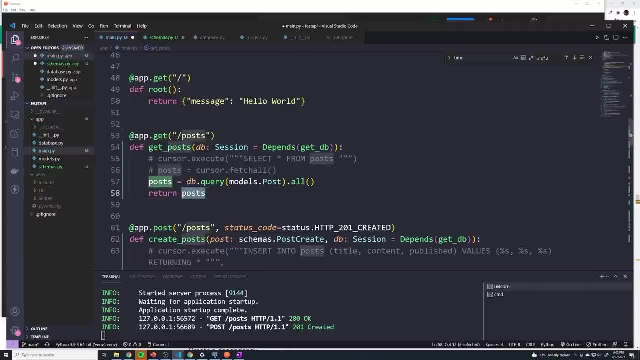 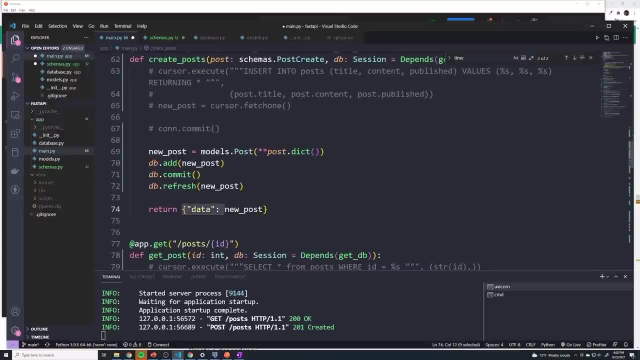 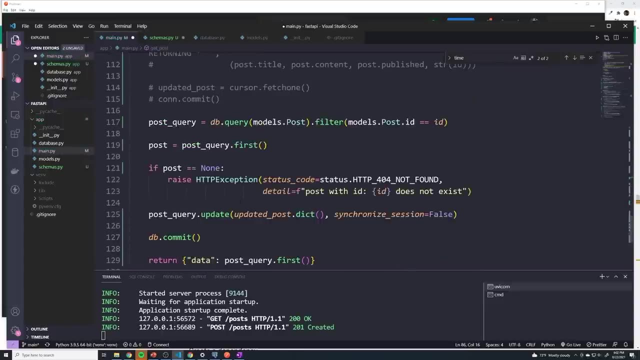 posts, And so it so fast. API will automatically be able to serialize that and convert that into JSON, And I'm going to do that for all of these. we're just going to remove that data keyword for all of them. We don't need to do it for delete, but we do need to do it for update. 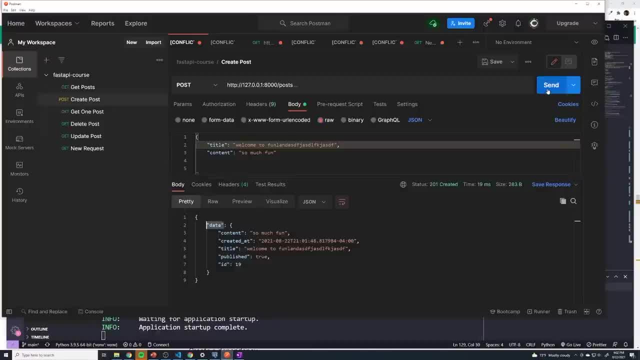 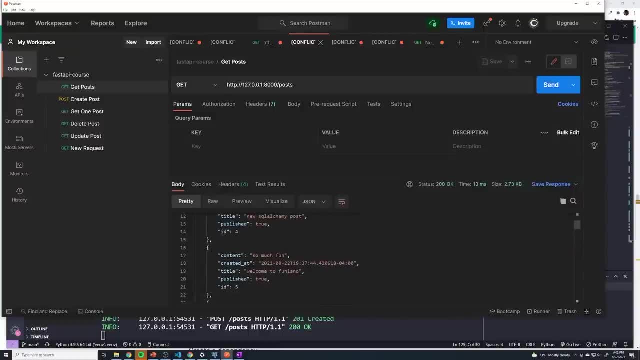 And so now, if we actually take a look at what this is going to look like, I hit send, you can see we just get back the post and we don't get that data keyword. Same thing for get posts. What does that look like? Perfect, So we don't have the data keyword. Now let's actually define what the 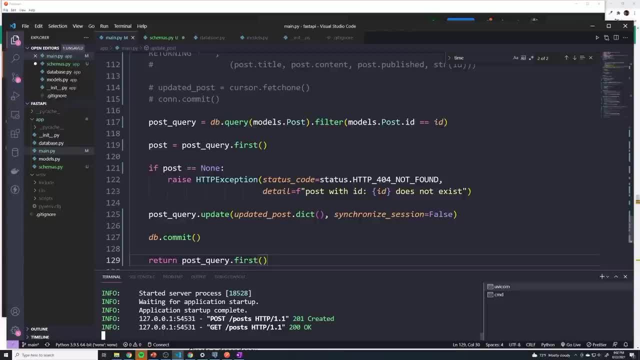 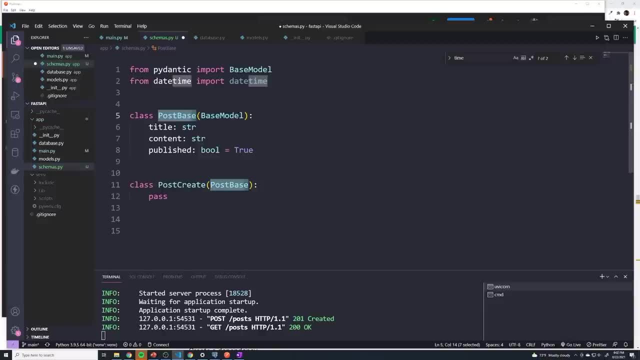 response should look like: And we do that with our schemas, we do that with our pydantic models, just like we have a pydantic model for creating posts which happens to just inherit from post base. So post create is just saying that we expect the title, we expect the content published. 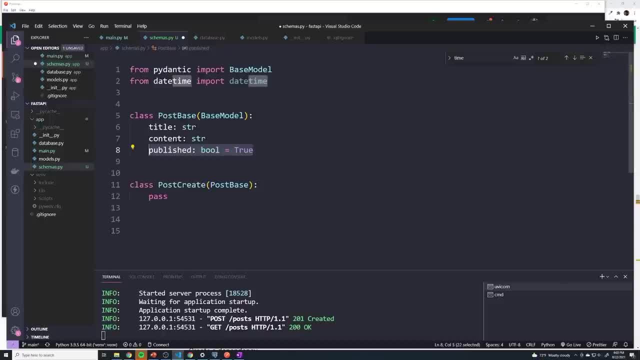 is optional, And if you don't provide one, it's true, And so we already know how to work with that. Let's create a brand new class for the response. So you know, this handles the direction of the user sending data to us, And now we want to handle us sending data to the user. So I can. 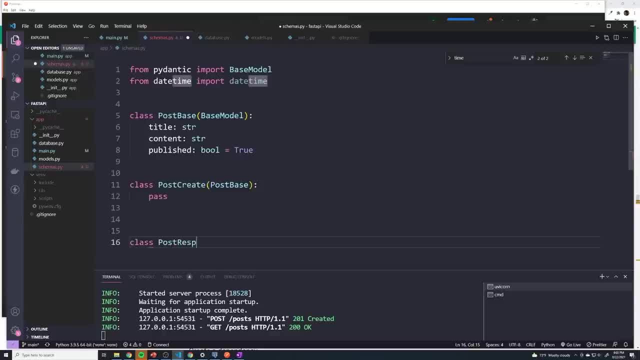 create a brand new class. we can call this post, response, or we, because it represents the response, or we can just call it post. it doesn't really matter, I'm going to call it just post. And then we're going to extend base model, because all of our pydantic models have to extend base model. 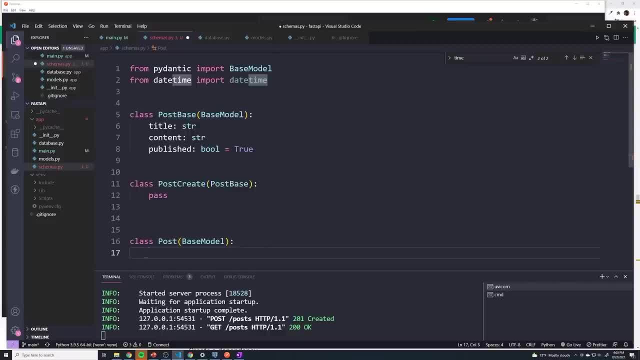 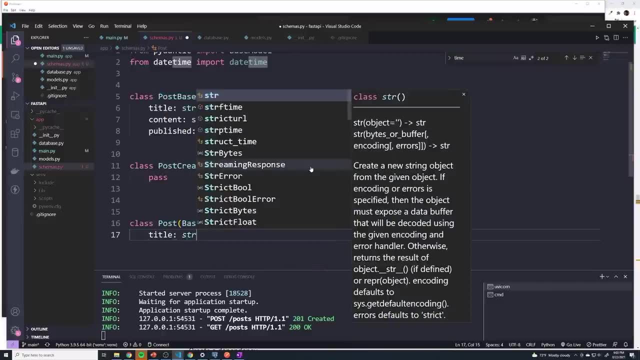 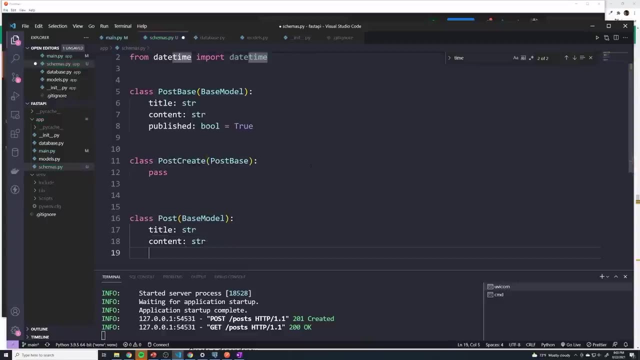 And then from here what we have to do is we have to specify all of the fields that we want in the response. So we want to send back the title, because that makes sense. So we'll send back the title, We'll send back the content, which is going to be of a type string, And then we'll send back. 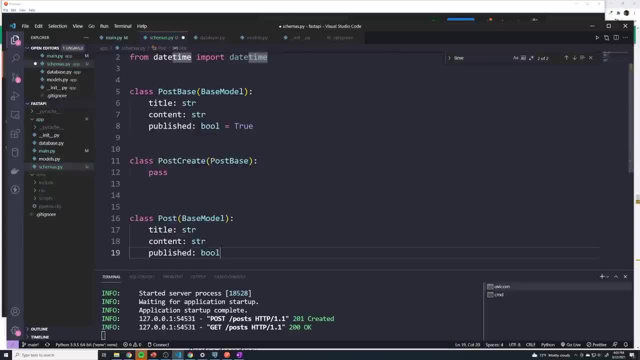 published as well, which is going to be a Boolean, And let's see what that looks like. Alright, so this still looks exactly the same as the other ones, But if you actually see right now, for any of the one requests that we sent, we get back the ID. 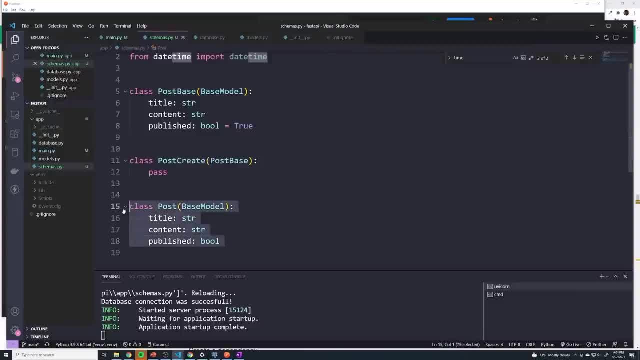 as well as the created at field. But since we didn't include those two fields, we shouldn't actually send it back to the user. So let's actually try this out. So I'm going to save this And then to actually define the response model. 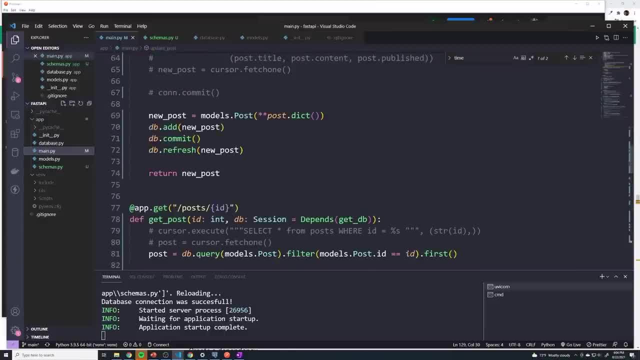 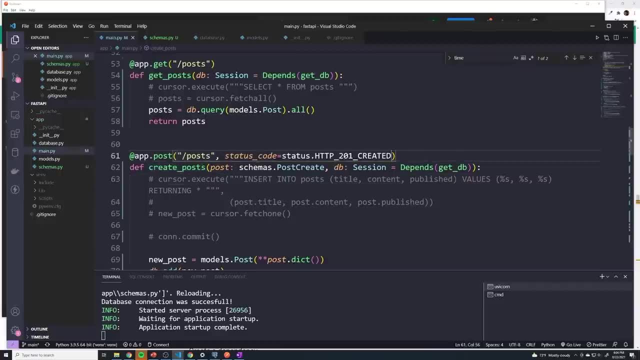 Under a specific request we'll start off with. we'll start off with the create request or create posts, And then within the decorator we just pass in another field And this is called response model, And then you can just let VS code automatically select it, And then here we just reference. 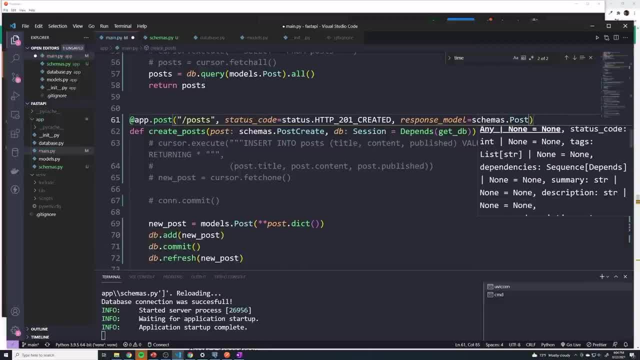 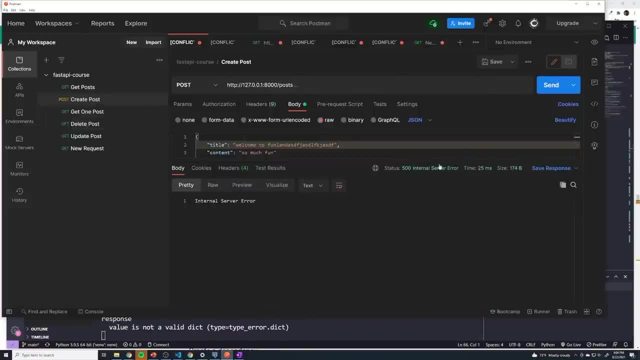 schemas, dot and then the name of the class. So let's try this out And let's see what happens. So now, if I create a post, we get a 500 error, And let's see what happened. It says value is not a. 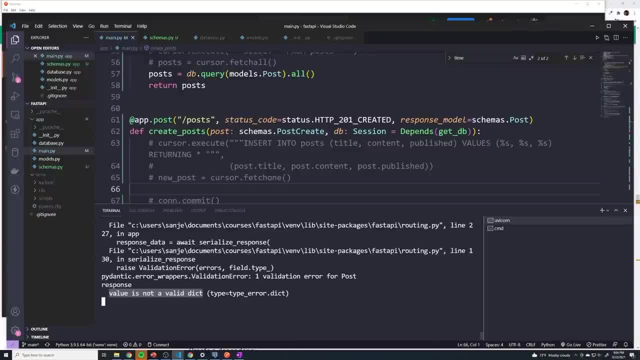 valid dict. So it's. it looks like pydantic is saying that. you know, when we try to send the response, the data we got back was not a valid dictionary right And because pydantic- the pydantic class, works with dictionary, takes a. 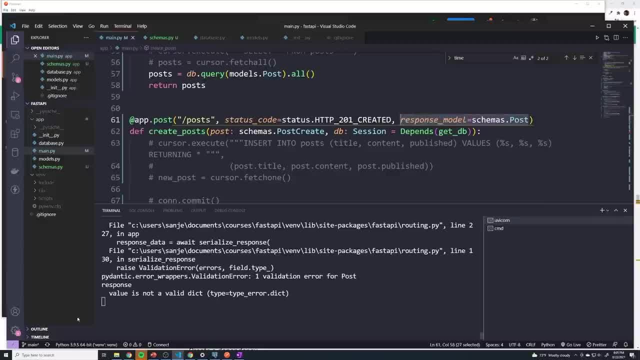 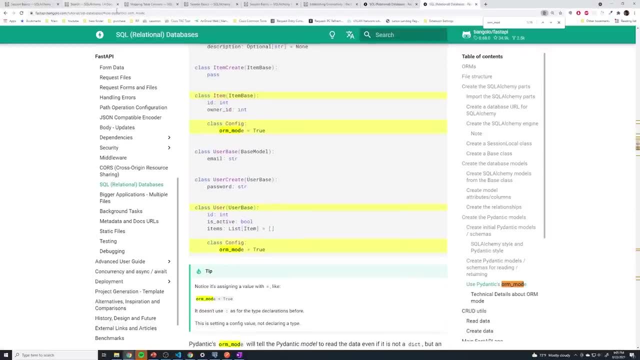 dictionary and then converts it to that specific model. So what exactly happened here? Why is this causing an error? Well, if you look at the documentation- and where is it right here, if you go under SQL relational database, it says that for your models, your pydantic models, we have to add: 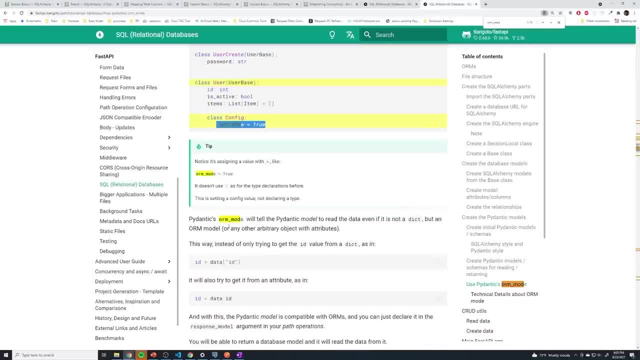 this extra config class, config or mo true, And explains exactly why we need that Right. Because, by default, the pydantic model will only read it if it's a dictionary right And that's what it's expecting in our code. because 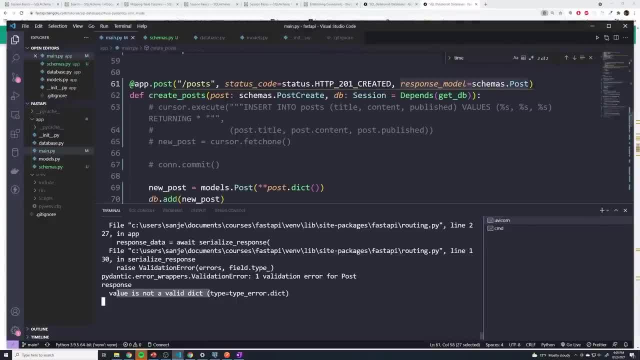 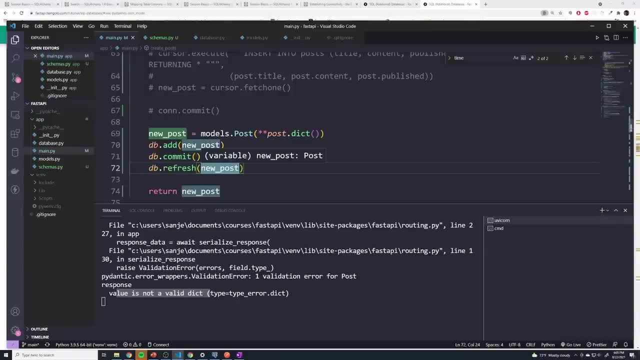 we see the error. it's not a valid dictionary, And that's because when we actually make this query, write new post. this is actually not a dictionary, it's a SQL alchemy model, And so pydantic has no idea what to do with the SQL alchemy model. it only knows how to work with dictionaries. So we have to. 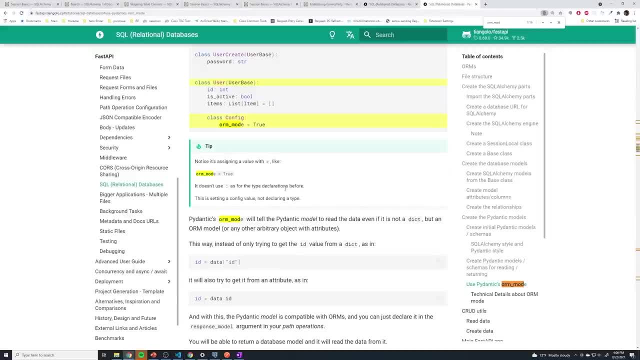 tell it to actually convert this SQL alchemy model to be a pydantic model, And we do that by passing in this specific text right here. So this is going to say, or mo: true, this is an ORM model and it's going. 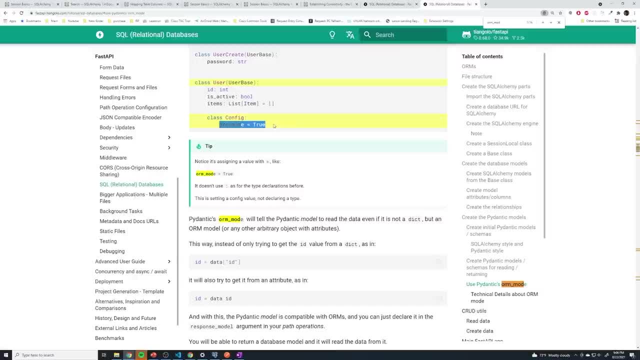 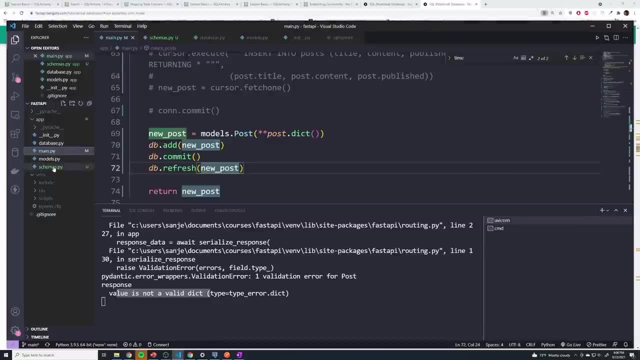 to tell pydantic say to: you know, ignore the fact that it's not dictionary and go ahead and convert it. So we can just copy this text and add this to our code for our post model, And that should be properly in there. 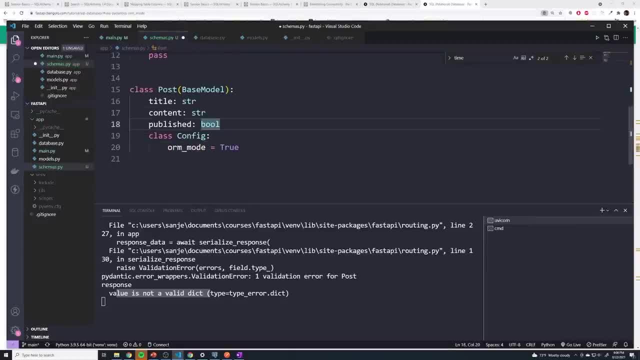 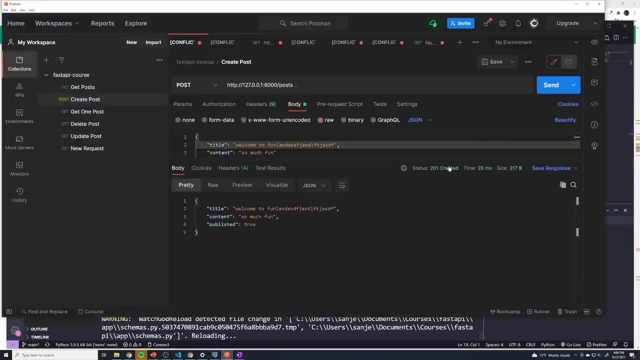 dented. Now that should be good And let's see if we still get an error. now Let's hit send. Look at that, we got it. it seems like everything worked Okay to one created. But take a look at the fields. 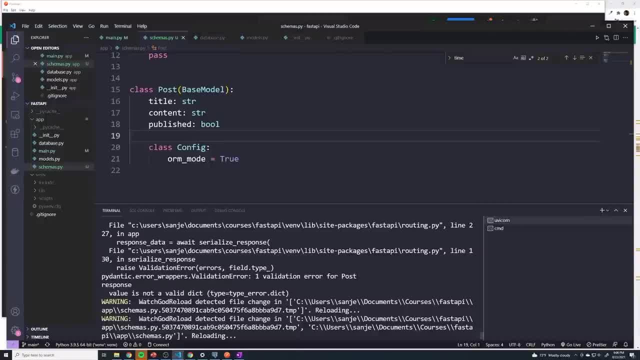 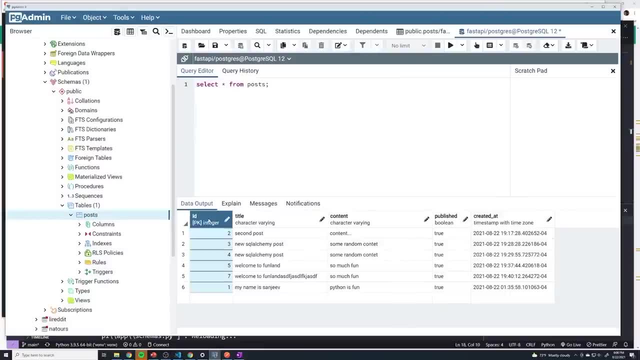 that we got back. we just got title content published And that's because our model is explicitly specified: title content published. Now we know, if we go to our Postgres database, we do have an ID field and it created that field. So if we wanted to add those, 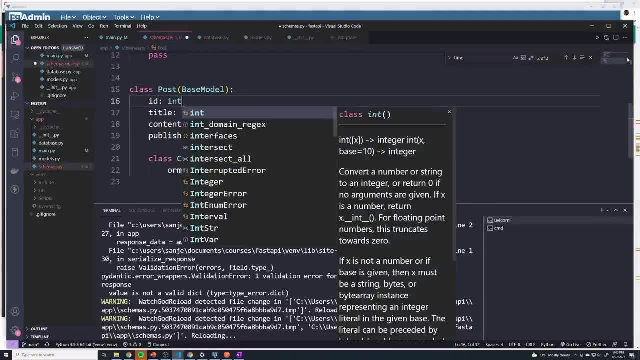 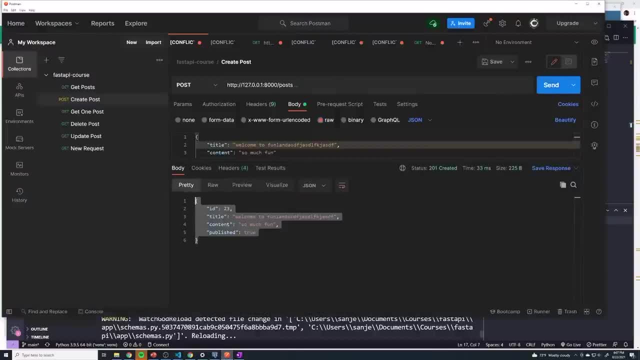 we can say: ID which is going to be of a type int. Let's save that And let's see what that looks like. Right now we get the ID back, Perfect. Well, do we want the created at time? I think you know. 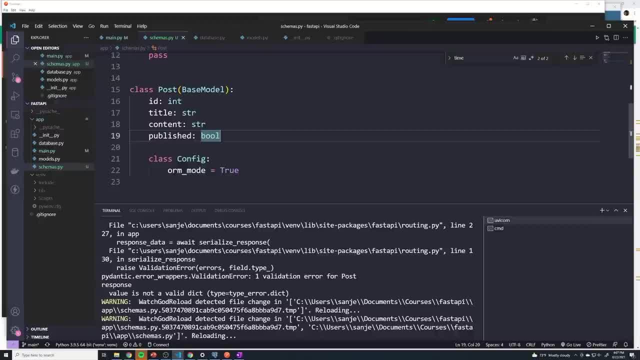 your front end code probably wants that as well, So let's go ahead and add that. So here we'll do: created at Now. what should the type for created at be right? it is ultimately, you know, a date and time. Well, 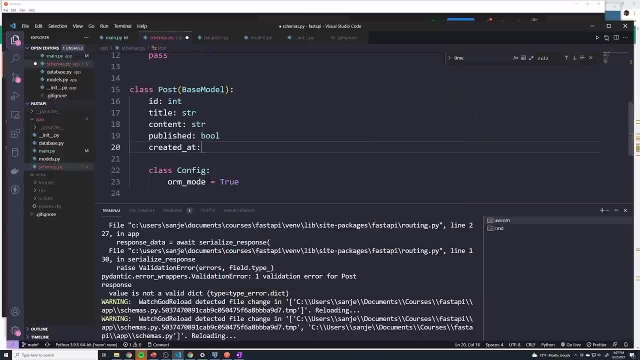 we can. we can do. you know something like this, You can pass it to. you know something like a string, But what we can do that's better than that, is we can import from datetime, import datetime, And so now we can say that the time 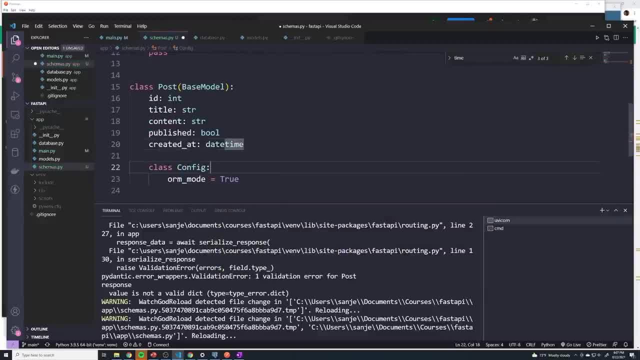 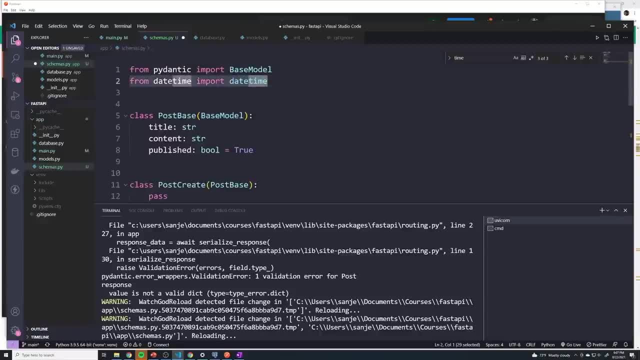 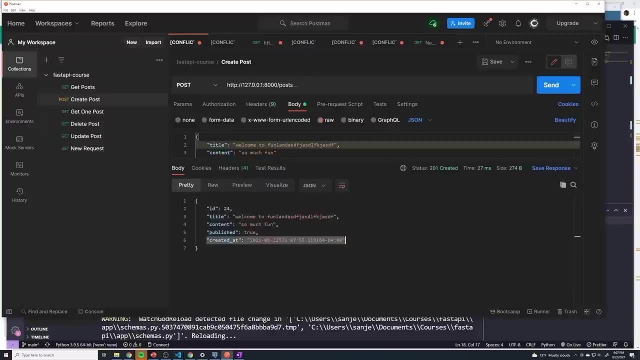 that created. it is going to be of type datetime, And so this is an extra little bit of validation to make sure that what we send back is a actual valid date time. Just make sure that you import it on in this file. And so now, if I send this back, we now get created at as well. So this is 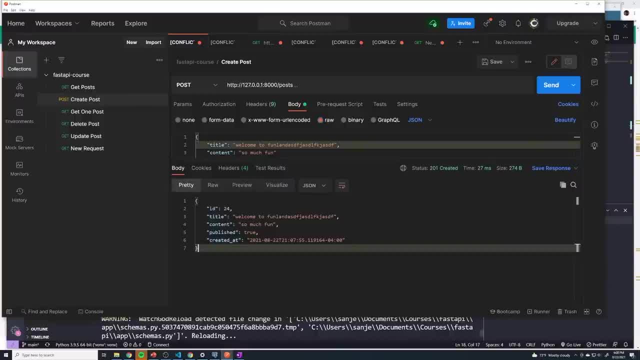 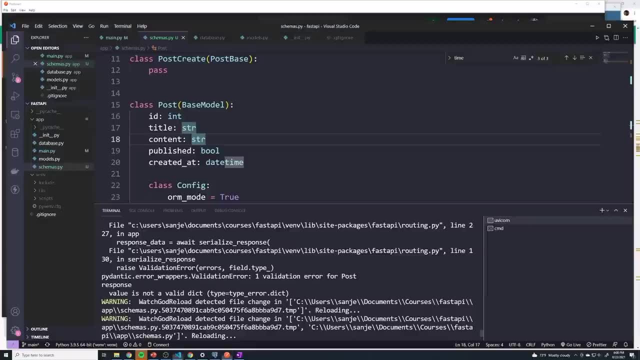 how we ultimately define the data that we send back. we can specify exactly the fields we want, And that way we can ensure we don't unnecessarily send data that shouldn't be getting sent Right. and we can do this with anything. I can just send back the ID if I really wanted to. 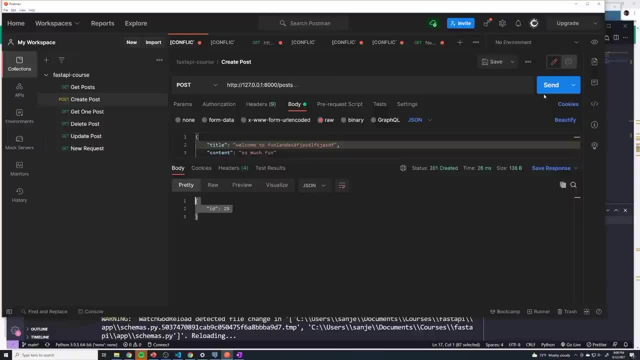 Now we just get the ID right. you see, there's a lot of flexibility and a lot of power when it comes to defining your responses, just like we had when it comes to defining our requests And with API's. like I always say, make sure you explicitly define the exact data you want. 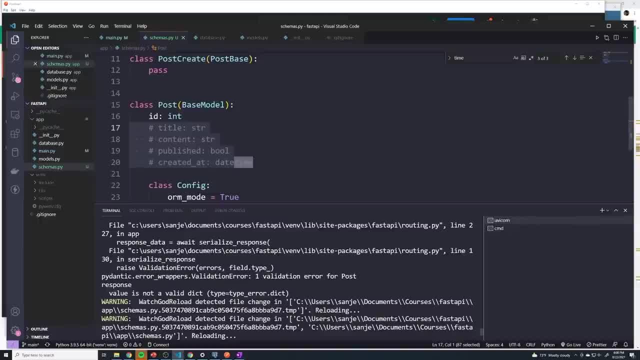 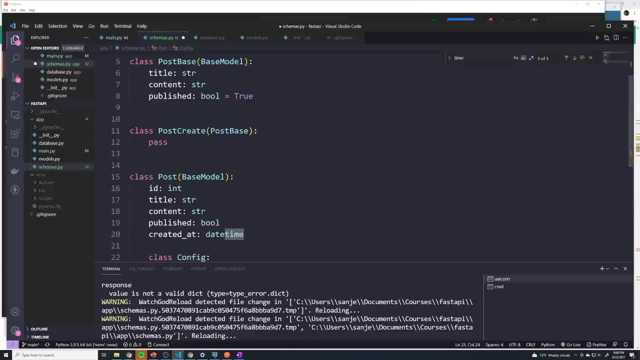 to receive and the exact data you want to send back to the client. Now, before we move any further and wrap up this video, you'll see that there's a lot of duplication, right, Because this post model for the response, right, it needs title content published and then we're just adding ID and 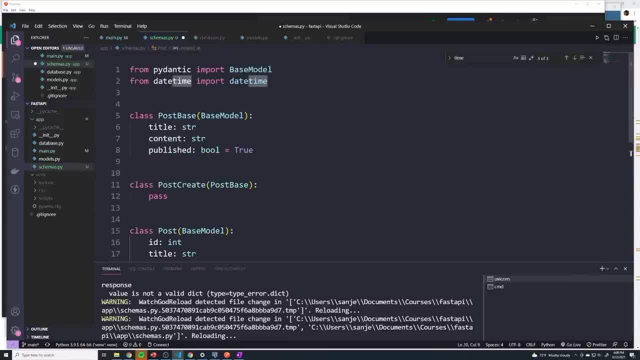 created at right And, like I said, when it comes to a real application, you're going to have so many more fields, so many more columns. it would be such a pain to have to repeat both of them, And so that's why I ultimately created this post base class, because 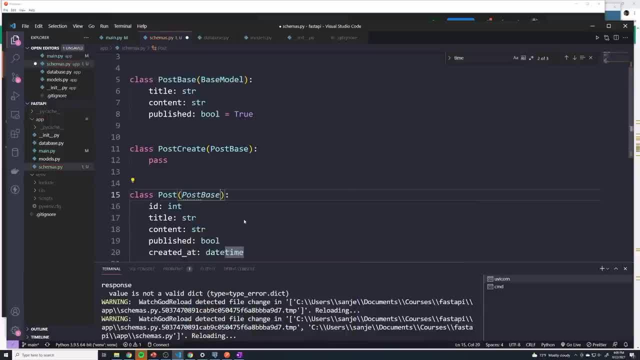 I can extend the post base class, And what that's going to do is that's going to cause me to inherit the title, content and publish fields, because they're already defined in here, And so I can just remove that, And so then I can just specify ID and created at. 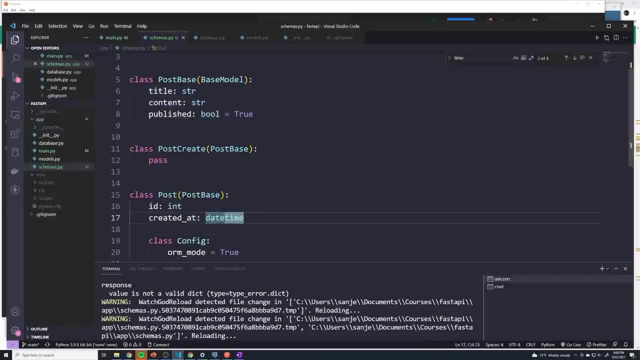 and then it's going to inherit the other three from the previous class, And so now, if I try this again, I send it. you can see that I get the same exact result. but I only had to specify the new columns I wanted to add in the response. 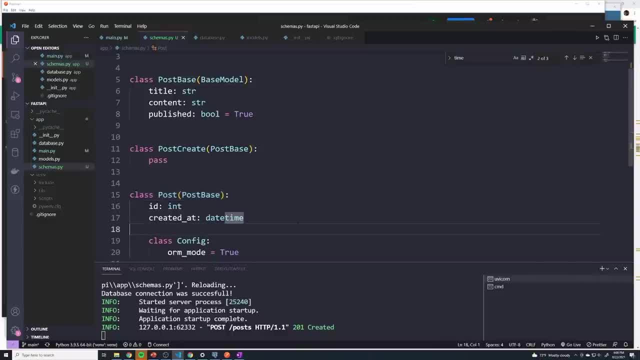 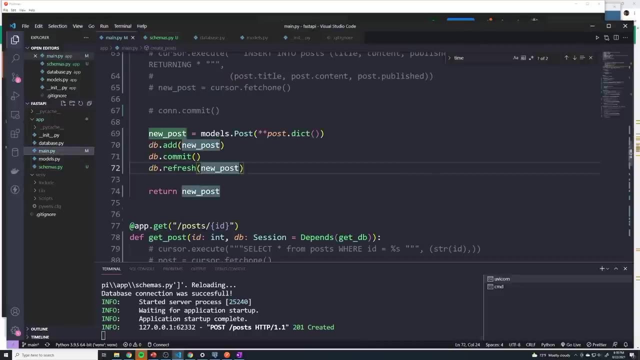 So this is really no different than, you know, working with any other model in Python. we get access to all of the usual features, like inheritance, so we can help reduce the amount of code that we actually write. Alright, and so now let's go ahead and update all of the other path. 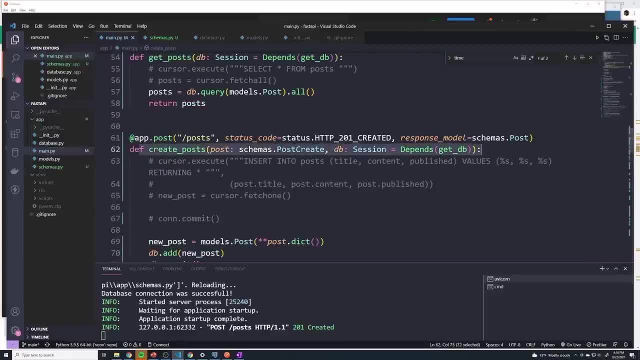 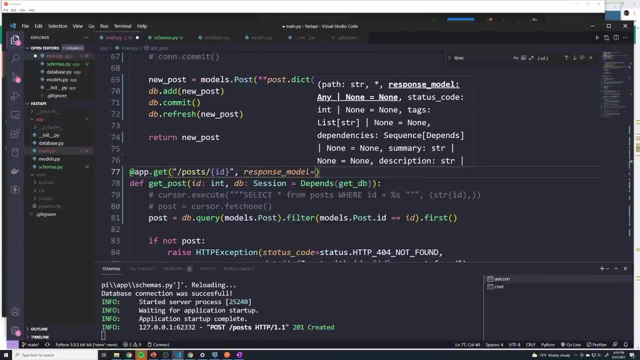 operations as well, because we can see that we only did it for create posts, But let's go ahead and do it for get an individual post. So there's going to be the same exact response model And we can just reference schemas, dot, post, And we'll do the same thing for our update post as. 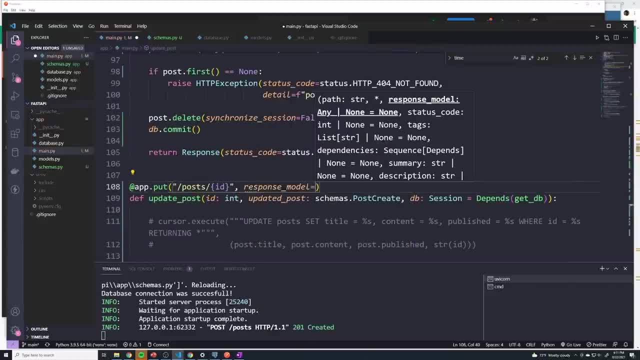 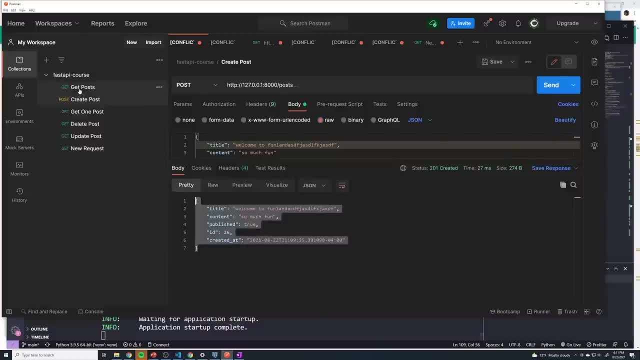 well, We'll say: response model equals schemas, dot post. And then let's just, you know, double check. So get one post. This, should you know we're going to go ahead and do that. So get one post This should. 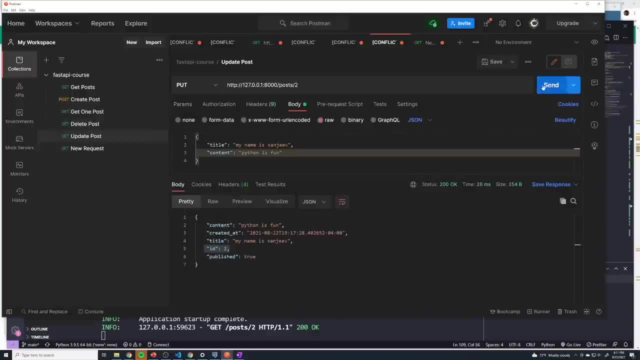 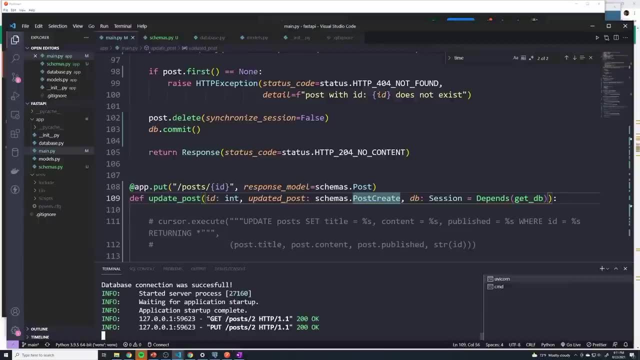 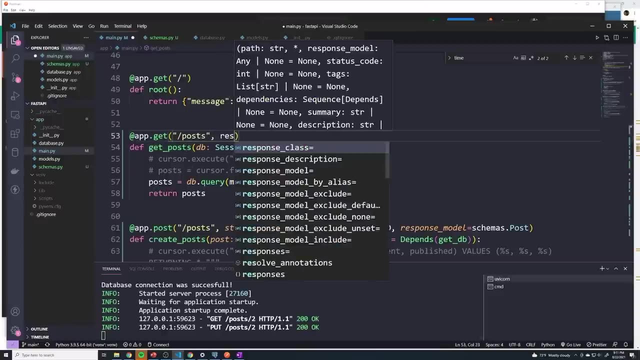 work just fine, perfect, And then update post And it looks like that works as well, And the last thing that we need to do is get all posts Right. So, right now, if we do get all posts now, where is that right here? we still haven't sent that, So let's do. response: model equals. 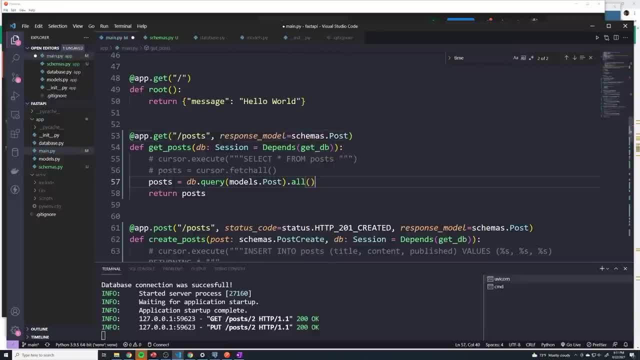 and then we can say schemas dot post. And then let's try that out. We hit send, we get an error, And this is expected. And I want you to stop and think about what exactly is happening, Because we are returning a list of posts. 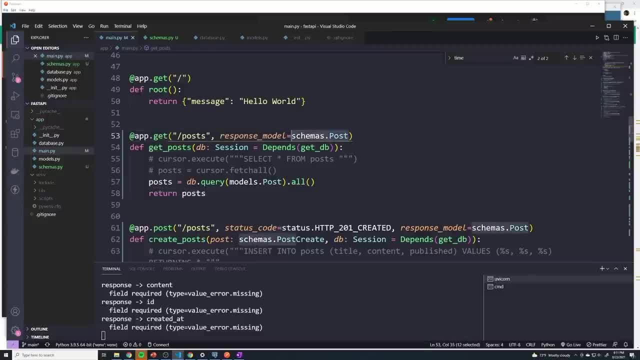 And it's trying to shape that into one individual post. We got a list of posts. We should be sending back a list of our schema post, So how do we do that? Can we just put a bracket or something like that? Will that work? 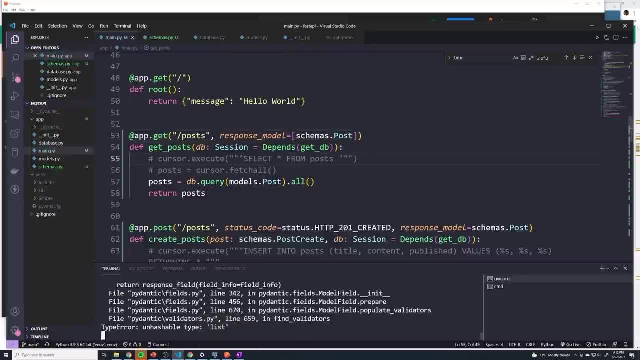 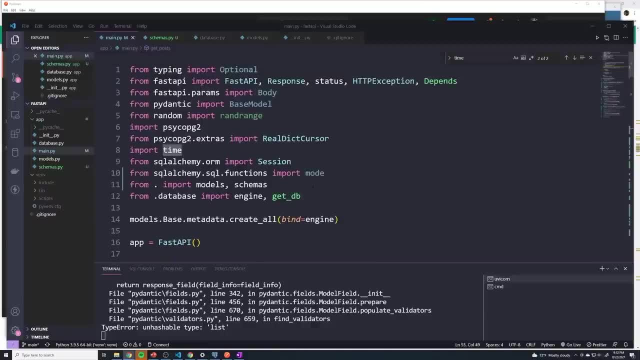 Let's try this. Well, it looks like there's an error, So this doesn't seem to work. So how can we specify? we want a list of posts. Well, we have to import something from the typing library. So we have an optional from the typing library. 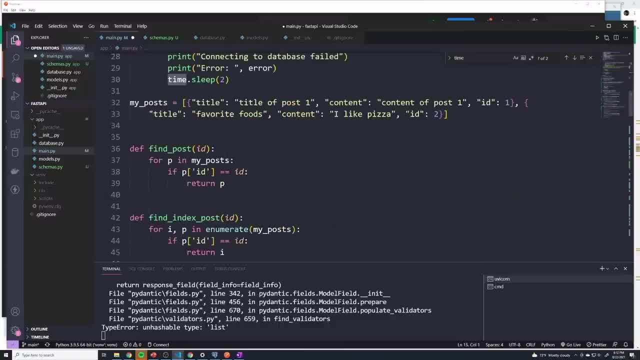 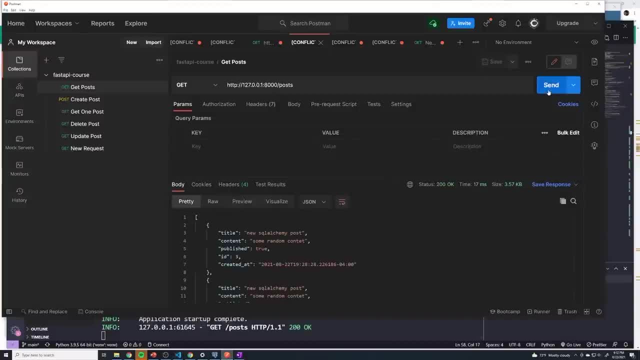 We can also import list. And so now I go back to our get posts, I can say list, And so now if I hit send, we should get back all of our posts. So here we're just specifying: we want a list of our specific schema. 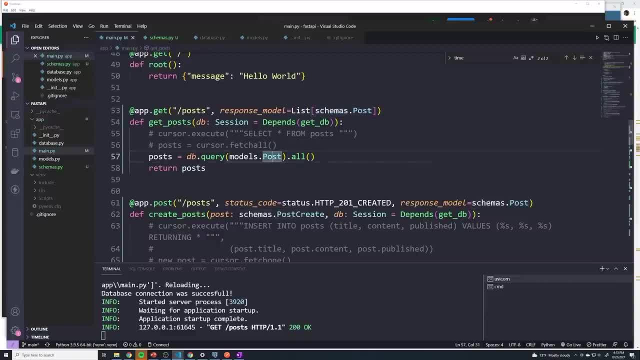 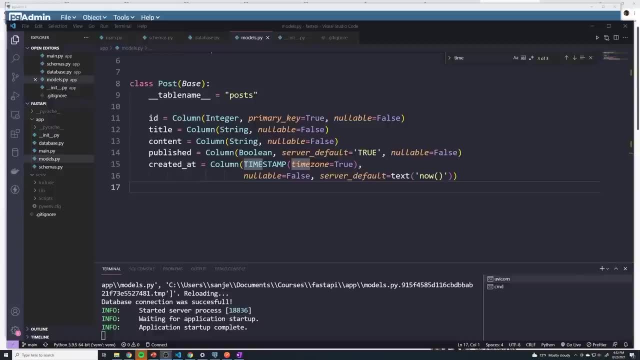 Schema post model, And that's just going to allow us to get a list of posts Very simple. In the next couple of sections, we're going to focus on creating user functionality, And what I mean by that is having users be able to actually 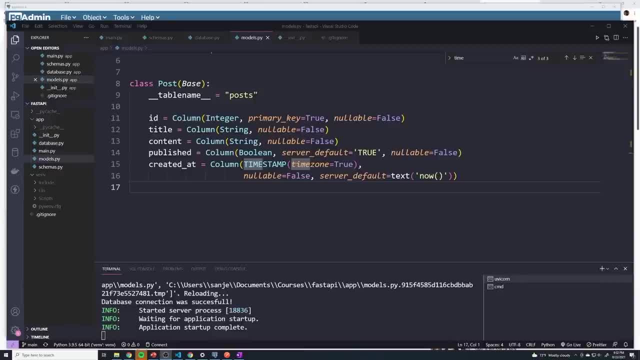 create an account within our app, being able to log in as well as being able to create posts that are associated with their specific account, And so the first thing that I want to tackle is handling user registration, So we need to be able to provide a way. 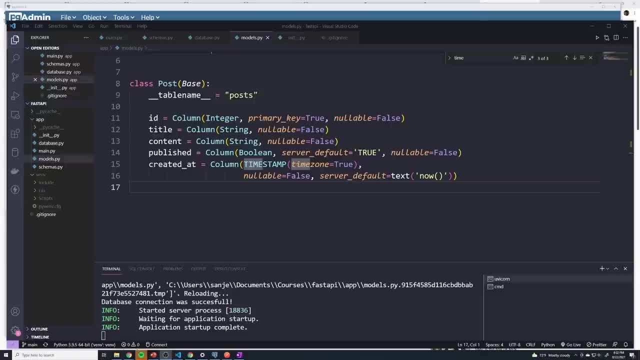 For users to create a brand new account, And the first thing that we have to do is we have to define our model or, more specifically, we have to create a table within our Postgres database that's going to hold all of our user information. 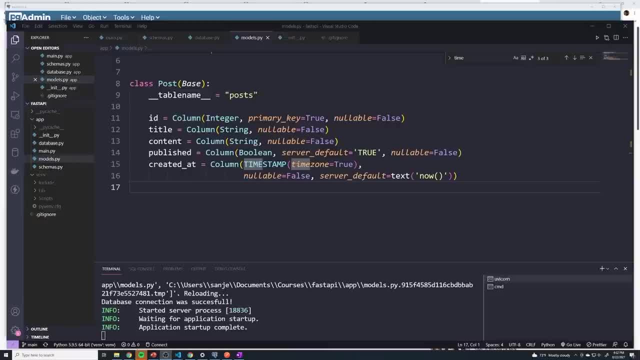 And so, since we're using SQL alchemy, we're going to create a new ORM model, just like we did for post, so that we can define what our Postgres table ultimately looks like. Let's create a new class, And I'm going to call this class user. 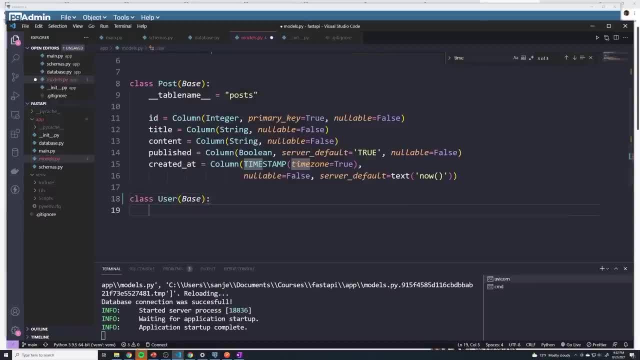 And this is going to extend base. That's just a Requirement for any SQL alchemy model. And then here we're going to provide the table name within Postgres. So I'm going to say the table within Postgres should be called. 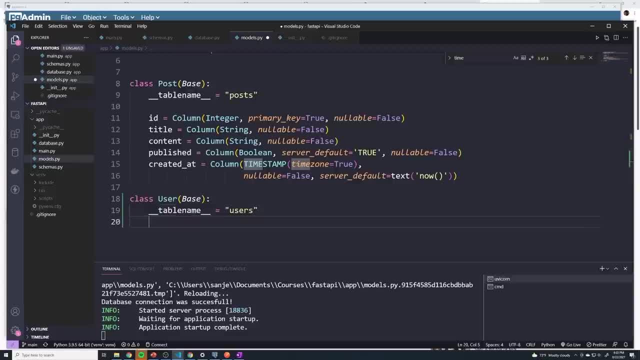 users, Then let's go ahead and figure out what are the different columns that we need, And so we're going to handle registration by having the user providing a email address, So we should have a column for us to be able to store their email. 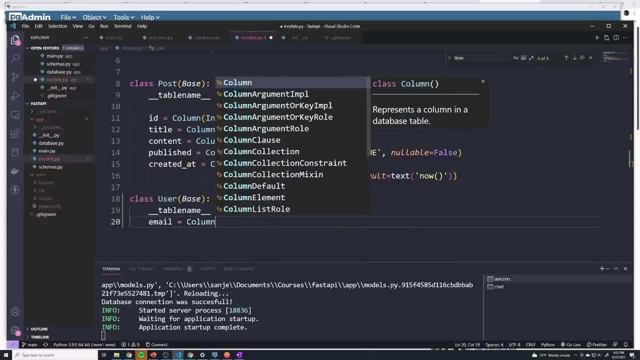 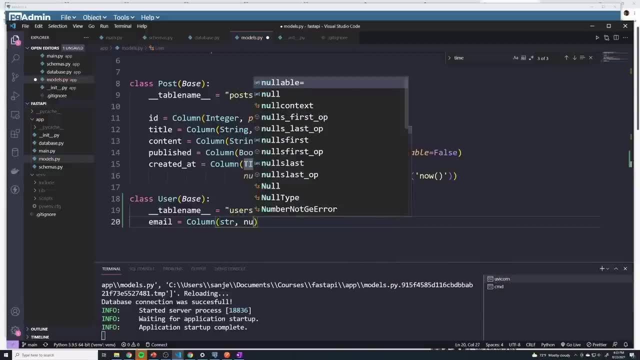 So we'll say: email equals column, this is going to be of a type string And we're going to say that this is nullable, is set to false, So they have to provide an email, And then, on top of that, we shouldn't allow someone within. 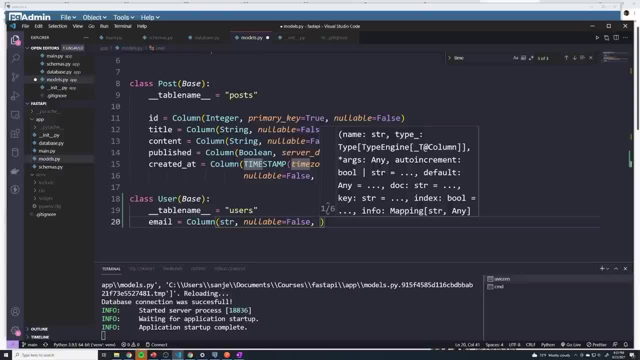 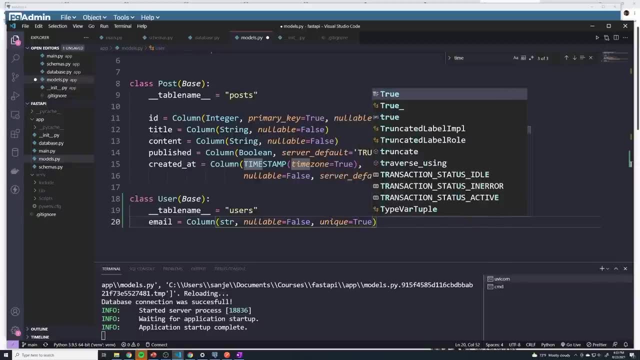 with a specific email to register twice with that email. right, there should only be one account with one specific email. So we're going to say that the unique constraint is set to true. That's going to prevent one email from registering to a password twice. 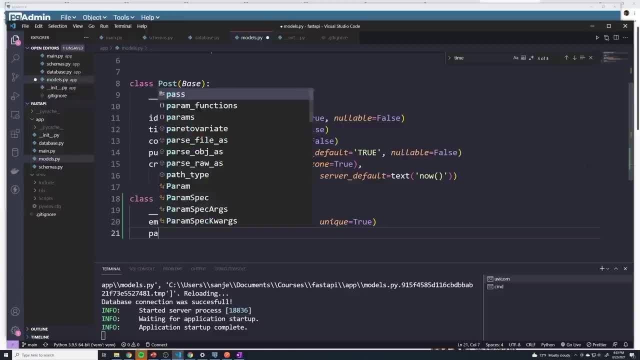 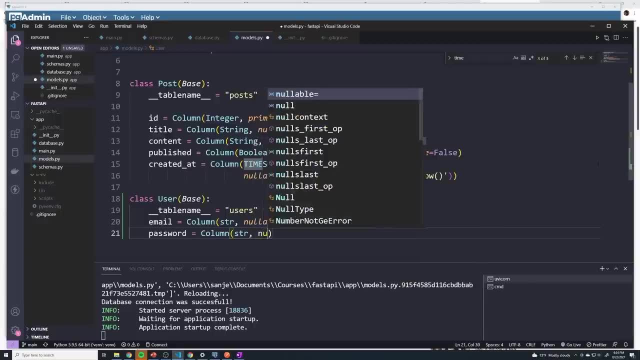 The next thing that we need is for us to be able to store the user's password, So we'll create a column for password. This is once again going to be a string, And then, once again, the nullable is going to be set to. 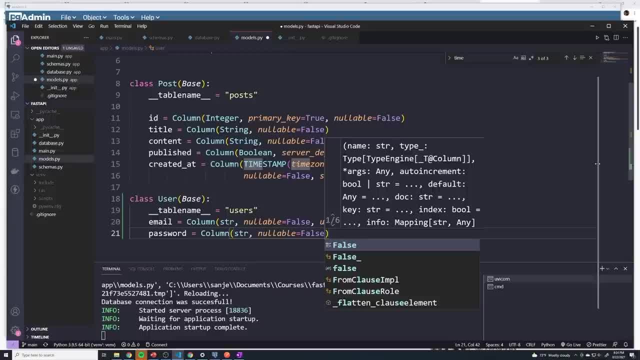 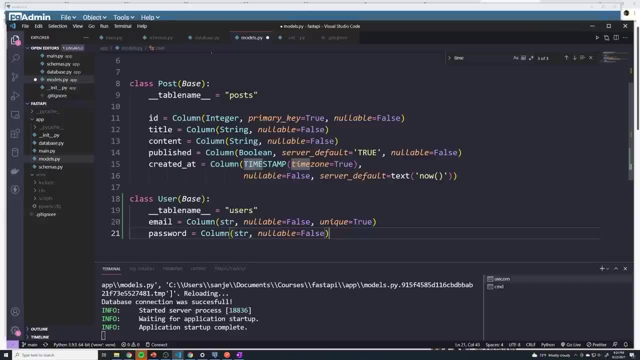 false, because we shouldn't be able to let them create an account without a password. And we don't need a unique constraint because I don't care if two users have the same password- it's up to them. And then finally, just like we had with the posts, 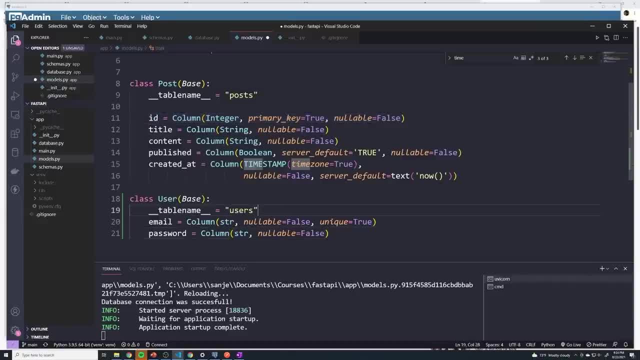 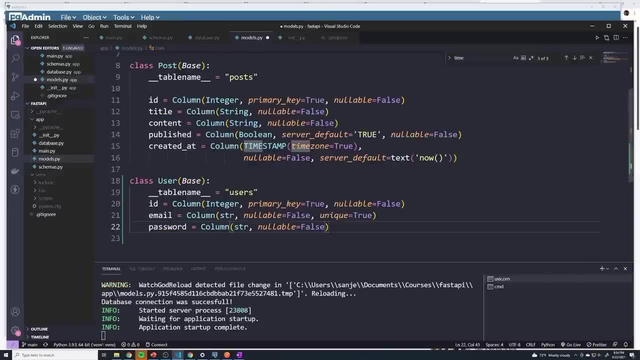 we're going to have a column for ID, So every user is going to have a unique ID. So I'm just going to copy and paste that, And so at this point, I think that's all we need for our user class. If you save it, it's going to reload the application. 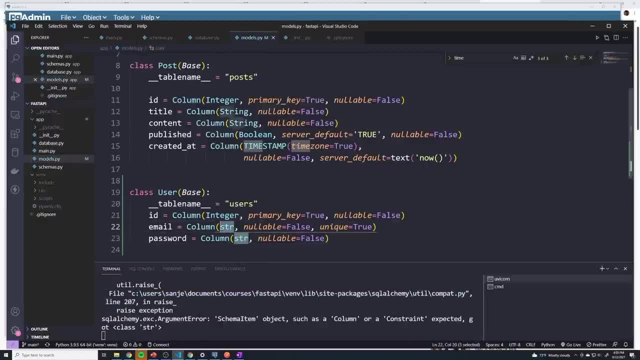 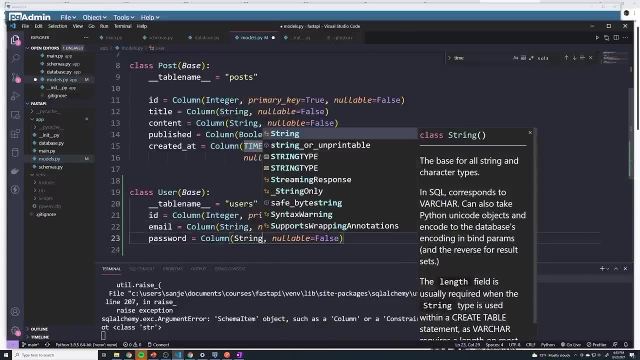 and it looks like I got an error And I realized this should not be STR, this should actually be string. That's my mistake. And then, actually, before we do anything else, I want to create it at column as well, So we can just copy this: 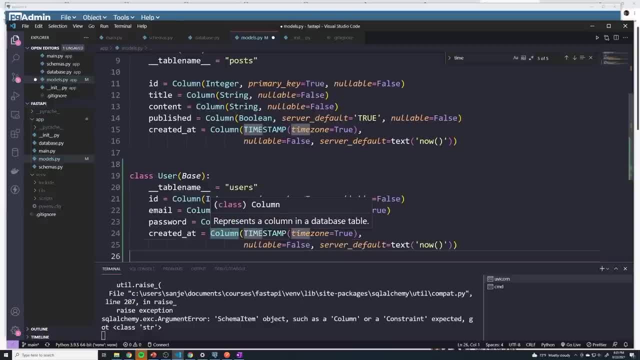 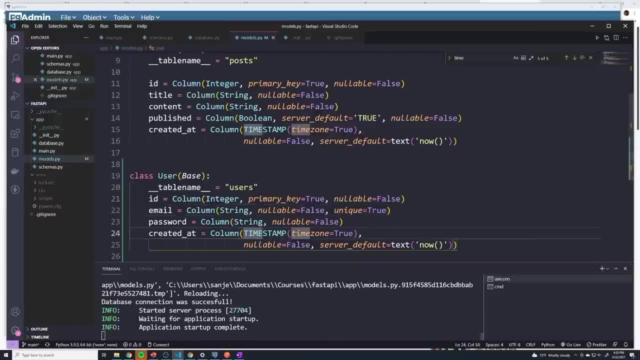 And then paste that in there. Like I said, pretty much anytime you create something in your database, you want to make sure that you record when it was created. you never know when you'll need that information, And so we've restarted our application. let's go to Postgres And under my tables. 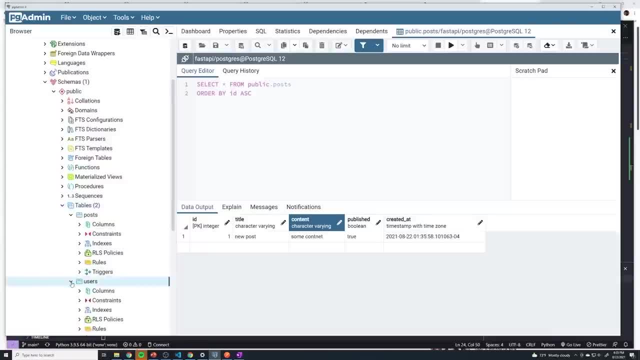 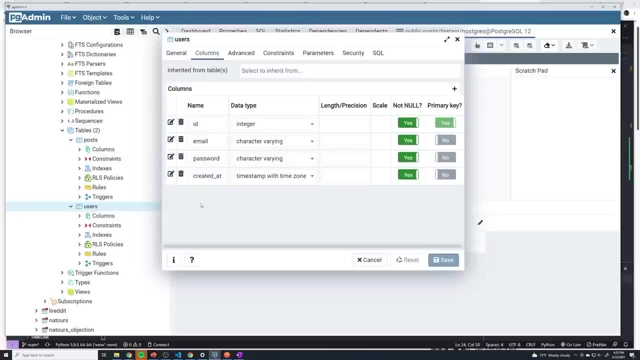 I'm just going to do a refresh And it looks like it went ahead and created our users table And if we do our users properties, we should see that it created all four columns and all of the necessary constraints should be set there. 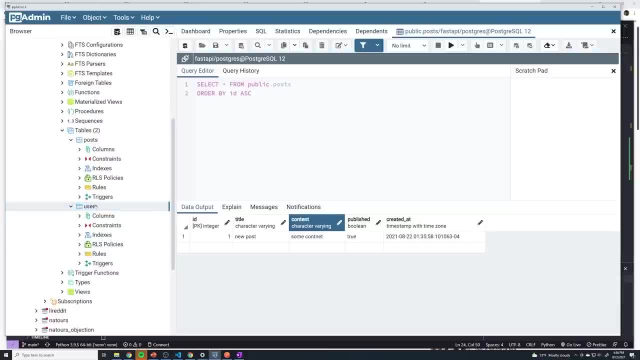 As well. And so let's, you know, just play around with this in Postgres just to make sure it works, Because I don't really trust SQL alchemy ever. So let's do right click And then we'll do view, edit data. So right now there shouldn't be any users. 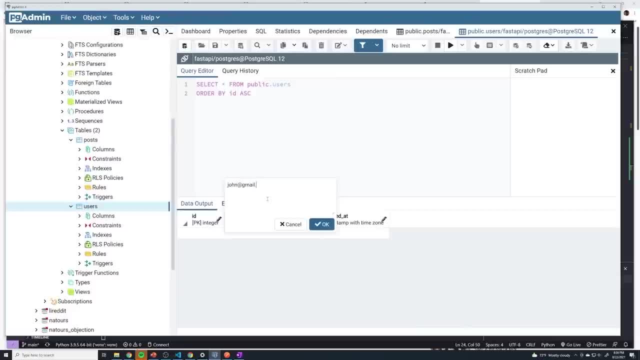 And let's create a new user. So I'll say: this is john at gmailcom password. you know, just put whatever you want for now And then, if we save that, it then successfully created a user. we got the generated ID as. 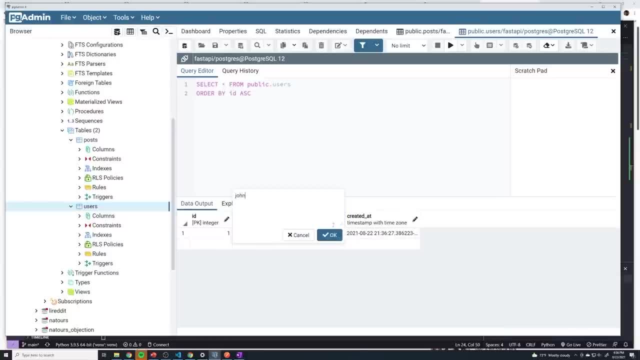 well as the created timestamp. And then let's create a new user. So I'm going to use the same exact email, So this should throw an error, because we shouldn't be able to register again. you know some random password, And then, if I try to, 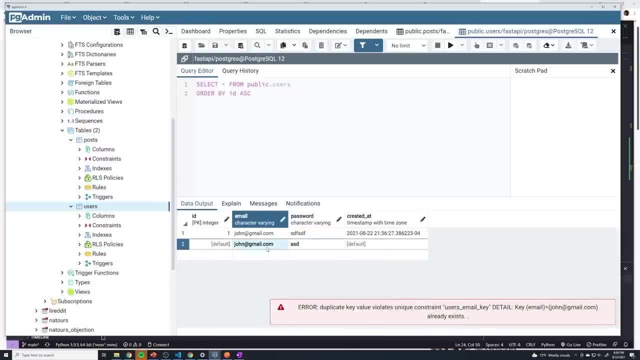 save this. we should get a unique constraint on users email error. So perfect, So that worked, And I'm just going to change this to be Cindy at gmailcom. We'll save that And it should create those users. So perfect, So we've got the first step done. when it. 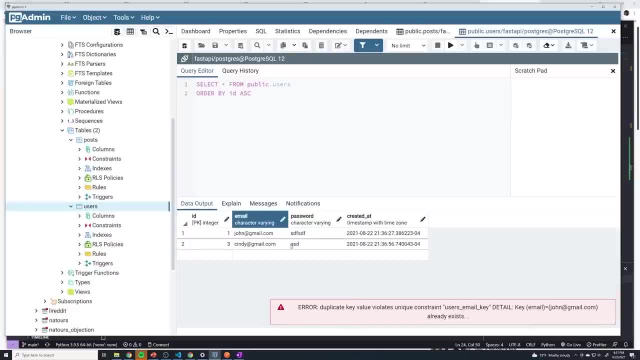 comes to defining our table. the next thing that I want to do is we will create a new path operation so that a user can actually send his username and password to our API, And then we can actually generate that user, Just like we did with posts. 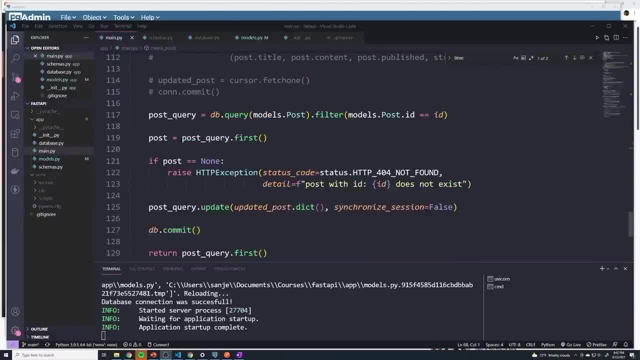 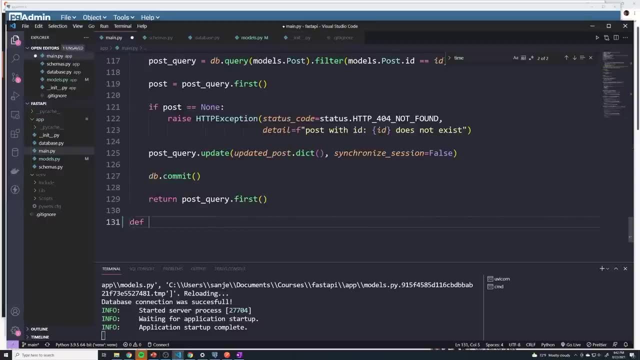 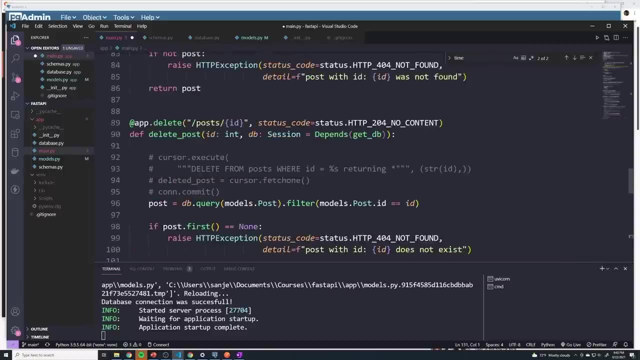 we're going to create a new path operation for creating a new user. So we'll go to the bottom of our main document And I'm going to create a new function. I'll say we'll call this create user, And so just like we have for. 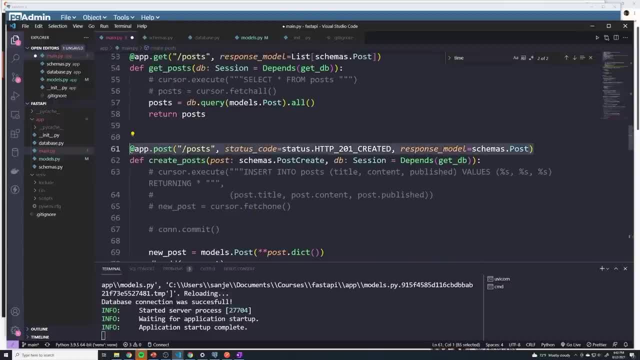 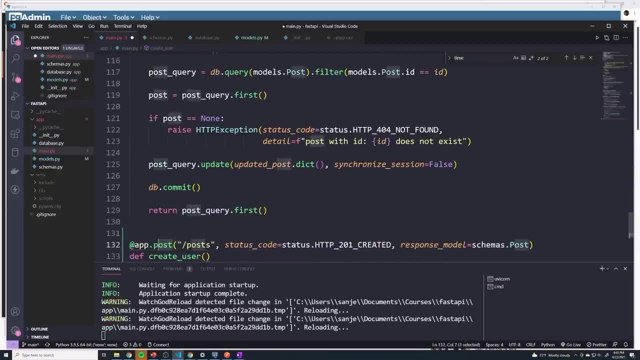 creating a post. I'm going to copy this decorator And we'll rename it, So it is going to be a post request, but it's going to be sent to the URL of users because we're no longer working with posts and, keep in mind, you get to select whatever URL or 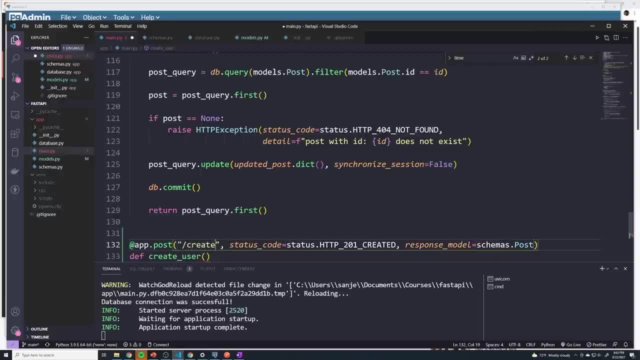 path you want to use. If you want to call this, I mean it's bad practice to call it create user, But you can choose whatever you want. I think it makes sense to call it users And anytime you create something, remember. 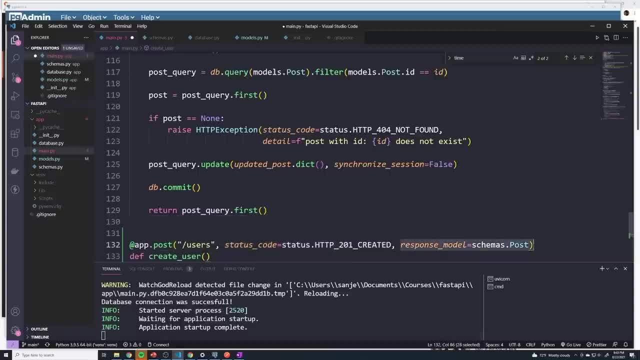 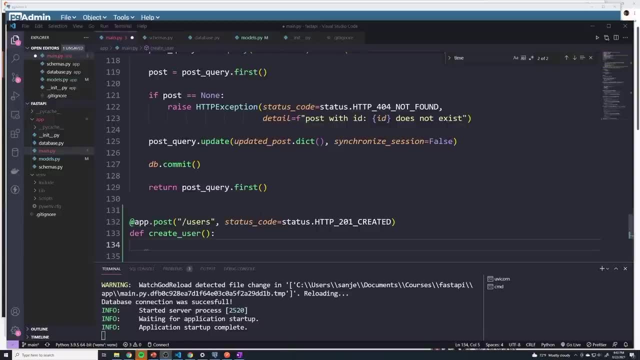 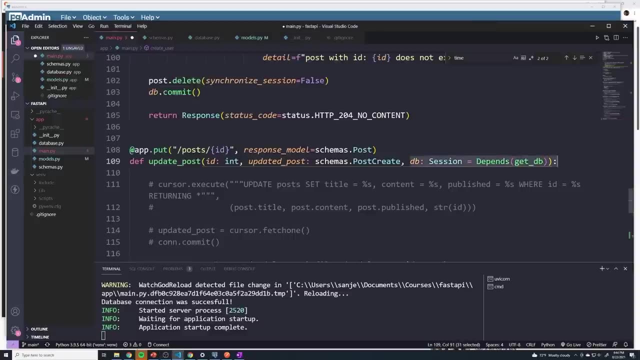 the status code should always be the default 201.. And I'll get rid of the response model for now, just to keep things simple. Now we're ultimately going to be using our database to create a brand new user, So let's go ahead and copy this DB right here from all of the 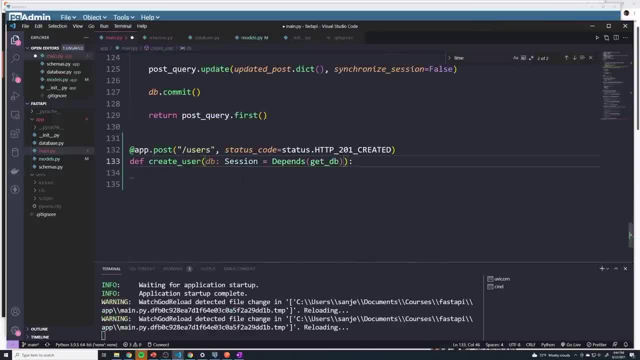 other path operations, because that's going to have to go in there And then, anytime we want to, you know, receive data from the user, because the user is going to have to send the email he wants to register with, as well as his password, in the body of the request. 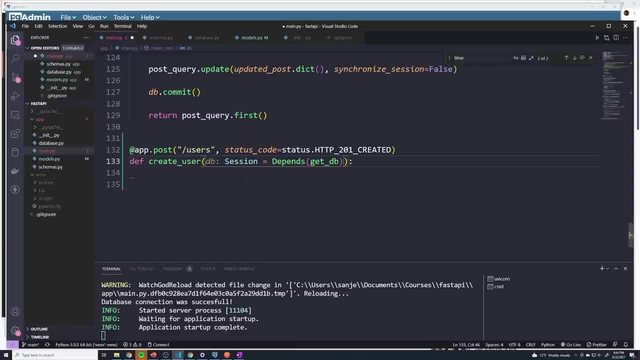 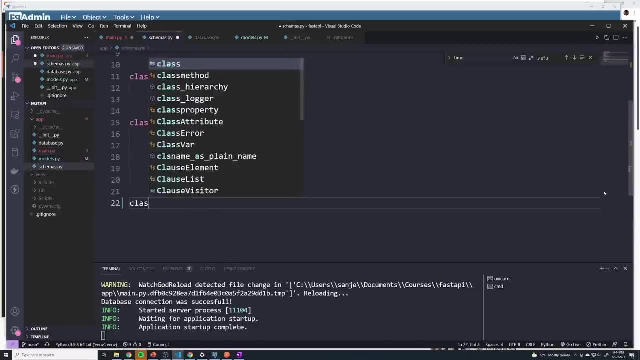 it always makes sense to define a specific schema so that we can ensure that the user does provide both of those. So, just like we did with posts, we're going to create a brand new schema And I can call this user, We can call this user, I think, this one it makes sense to call this user create. So this. 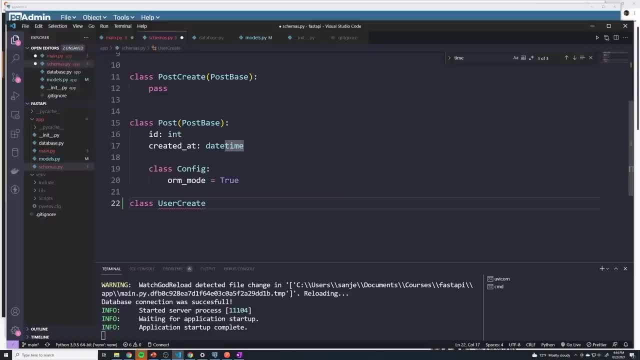 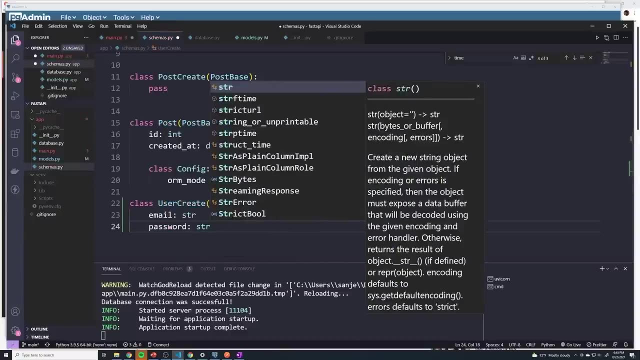 is going to handle just for creating users, And we're going to inherit from base model And for the user create, there's going to be an email field, which is going to be a string, as well as a password field, which is going to be of a type string And when. 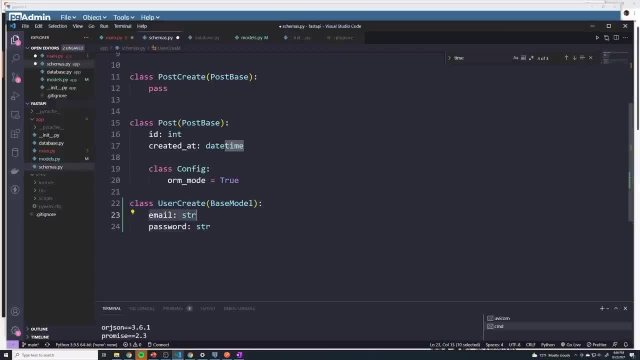 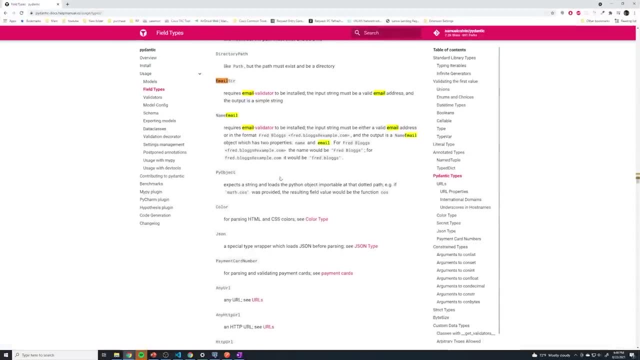 it comes to validating the user right, it's going to check to make sure that an email is provided. However, we can get a little bit more granular than that If you actually go to the pydantic documentation. we also have a field called email string. So this is going to validate. 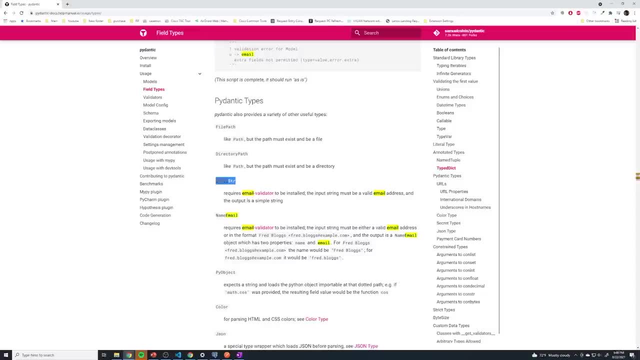 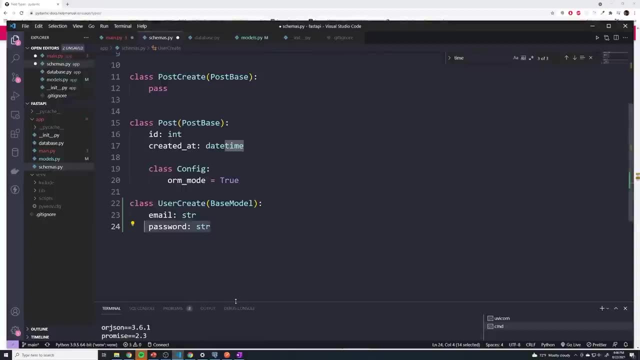 that the email property is a valid email. However, we need to have the email validator library installed, But that should automatically have already been installed for us when we installed fast API with the all flag, And so if you do a pip freeze, we should be able. 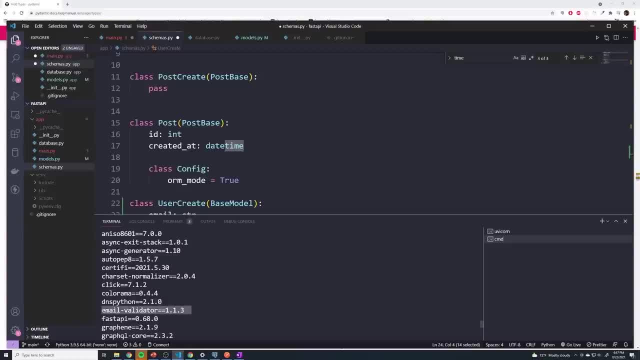 to see that we have a valid email. We should be able to see that we have a valid email. We should be able to see that we have our email validator already installed. If you don't have it installed for some reason, just go ahead and do a pip: install email validator. 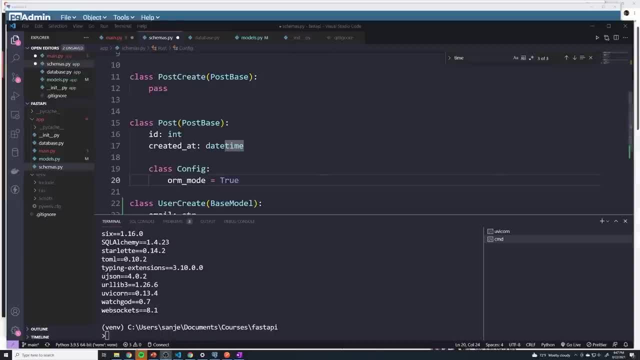 And that should install that library. And so what we'll do is, from the pydantic library, we're going to import email string And then we can say: this is going to be email of type email string that's going to ensure that this is a valid email and not just some random. 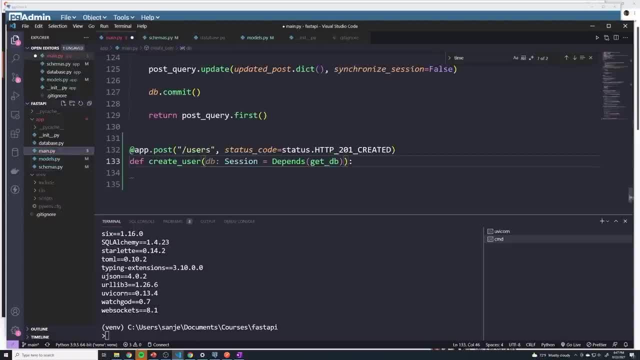 text. Okay, Then back in our main dot py file, Just like we did before, we can say user, and this is going to use schemas, dot user create, And so the email address and the password is going to be stored in an object called user. there's going to be a pydantic object as well, And 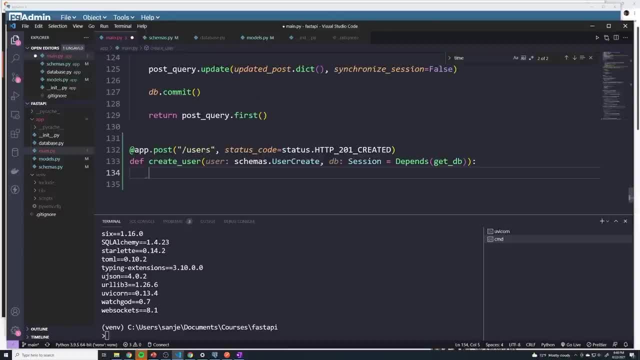 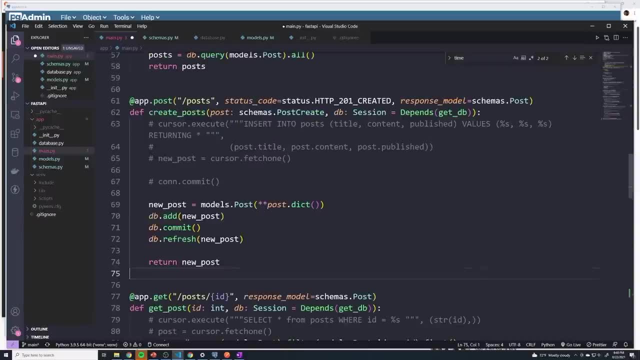 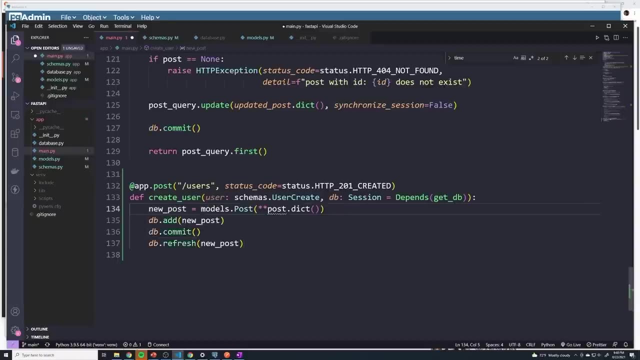 if you forgot how to save data to the database or create something with SQL alchemy, just go ahead and do that. So let me just go ahead and take a look at the Create posts And we can essentially just copy this And we're just going to rename a few things. We'll say new user And then 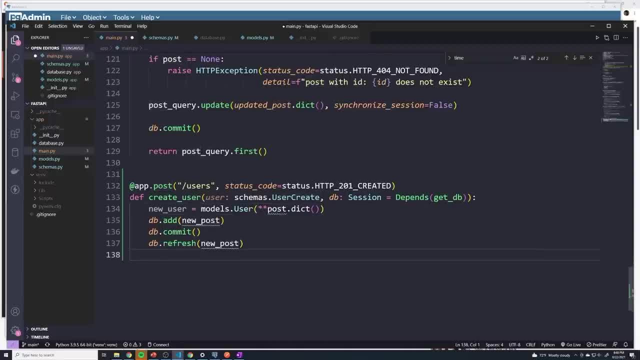 we're going to grab models dot user now And then once again. what we want to do is we want to take the user that we get back from here, from our schema, we want to convert it to a dictionary and then unpack that dictionary. 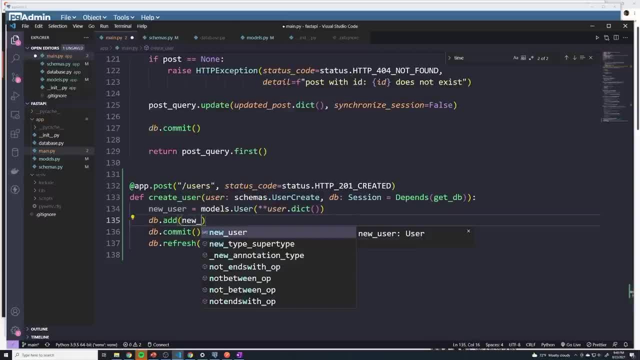 Then we're going to add it to our database, We're going to commit it, then we're going to refresh it So we see the brand new user, And then we can go ahead and just return new user. All right, let's give that a shot. And then, within our postman, we can right click. 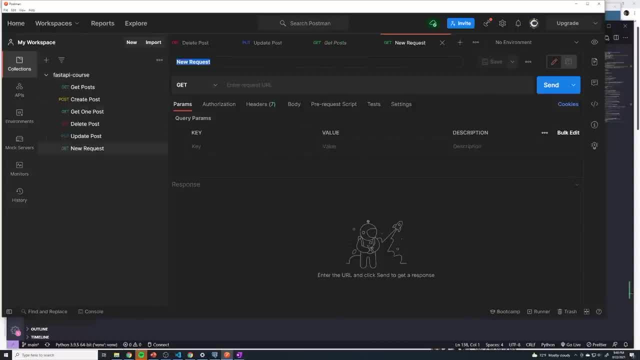 on this: select, Add request. we're going to name this: create user. This is going to be a post request, And then in the body we'll go to raw once again and then JSON, And then here we can pass in the email. We'll give it some random email, So I'll call this Carl. 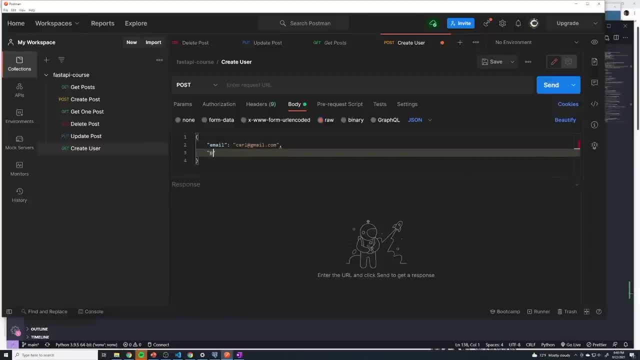 at gmailcom And then password. This will be password 123.. All right, and then we're going to go ahead and create a new user, And then we're going to go ahead and add a new user, All right, and then for the URL, just copy posts, And then here we'll just change this. 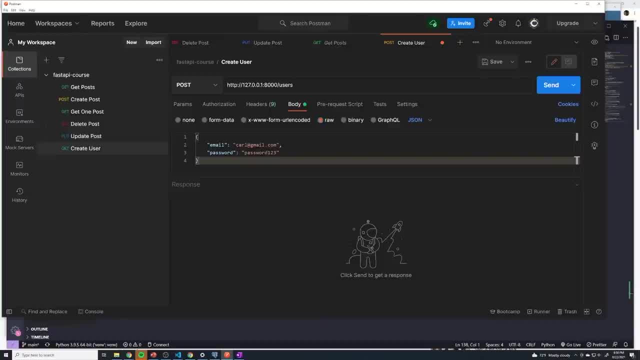 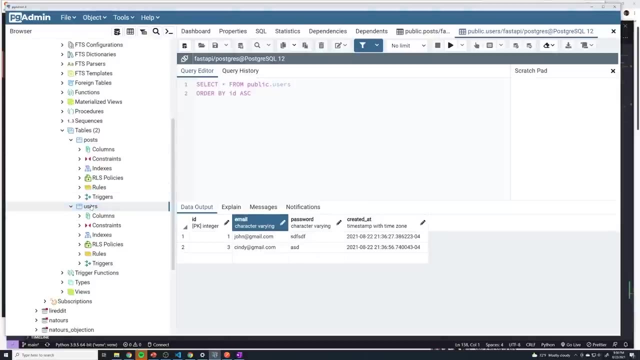 to users. All right, so let's give this a shot. Let's see if this works. And it looks like it worked right. We got the email, we got the password back, we got the created at and we've got an ID. But just to double check, like we always do, go ahead and go. 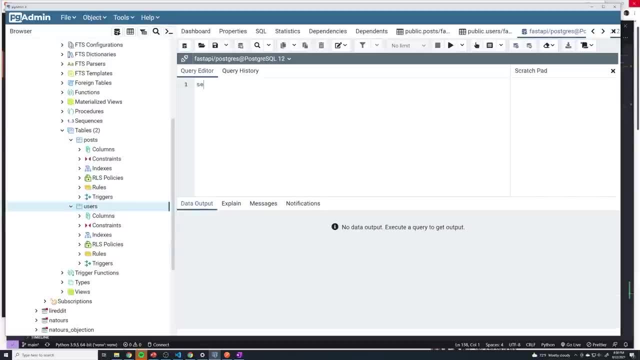 to your users table. select query tool, select star from users now, Because we're now querying no longer the post table, we're querying the users table. If I run this, we can see that we do get the new email that we created or the new user. 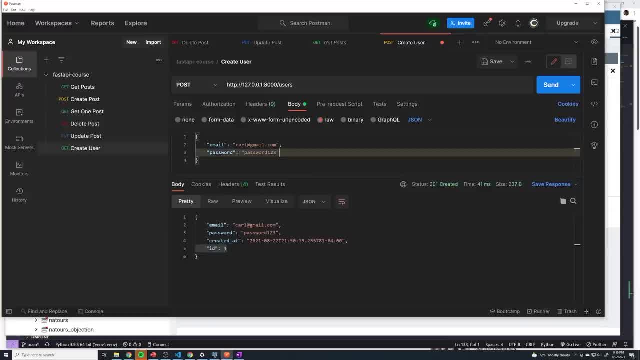 that we created with Carl at gmailcom. Now, as a quick test, just to make sure that email validator works, I'm going to change this And we'll just say some random txt: this is obviously not a valid email, So let's see if it properly creates that user And it looks. 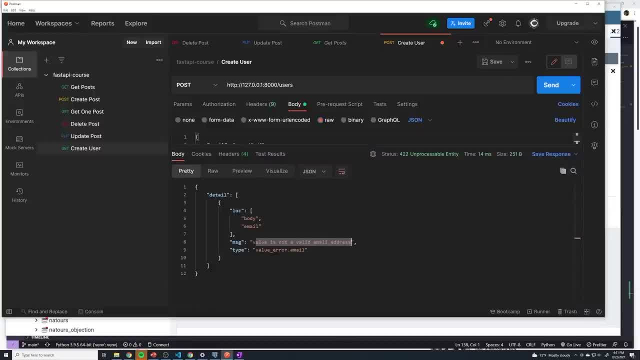 like, our schema validator worked and says value is not a valid email adress. So now we can create this new user And that's it. It works, Thanks for watching. and says value is not a valid email address. So you can see the powerfulness of the pydentic. 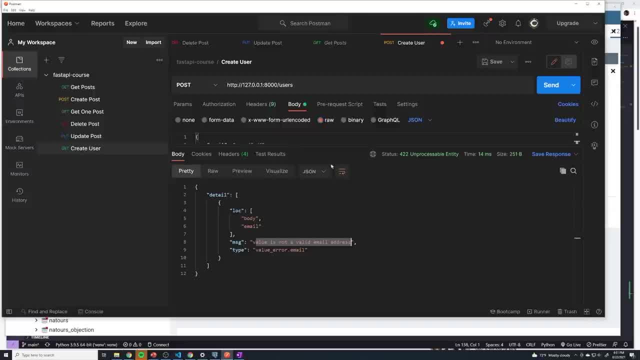 library, being able to automatically check to see if that's a valid email address, All right. But one thing I didn't like about creating the user is that if we change this back to a valid email, I'll say: just call this new user at gmailcom. We create that user. you see that he gets his. 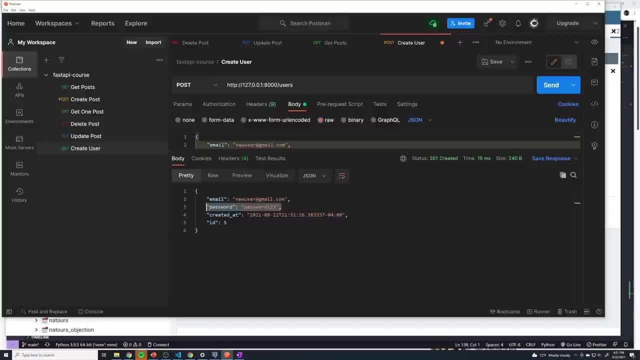 password back. Now why in the world would he want to see his password back? there's no reason to ever send the password back to the user at any point, And so one of the things I want to do is I want to define our response model so that we never send back the user, And I think you guys should. 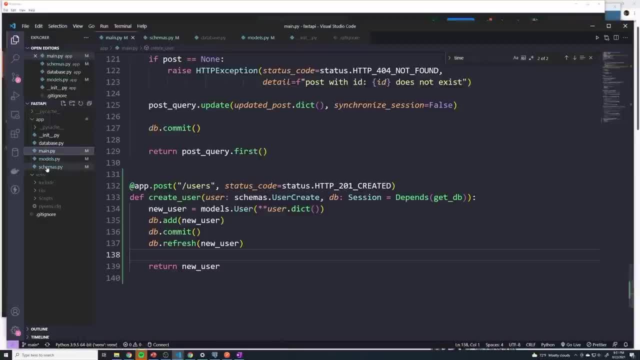 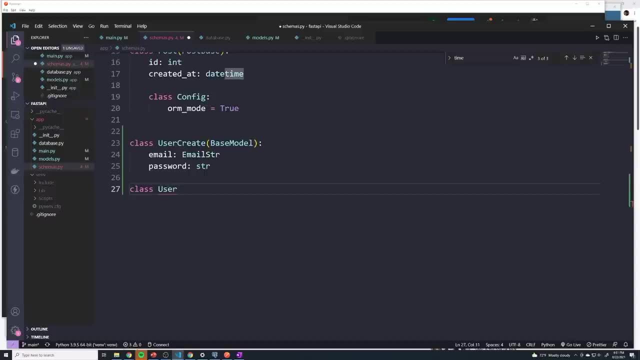 already be able to do that, But we'll walk. I'll walk you through how to do that. So let's go to our schemas. We've got our user create. let's create our, let's create a new class And I'll call this user out. And so this is going to be the shape of our model when we send back the user. 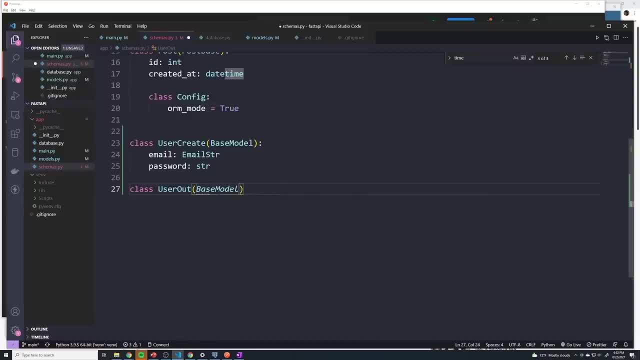 to the client that requested it. It's gonna extend base model as well, And here we're going to send out a couple things. So there's going to be an ID. now the user should know his ID email. that's going to be of email string again, And then 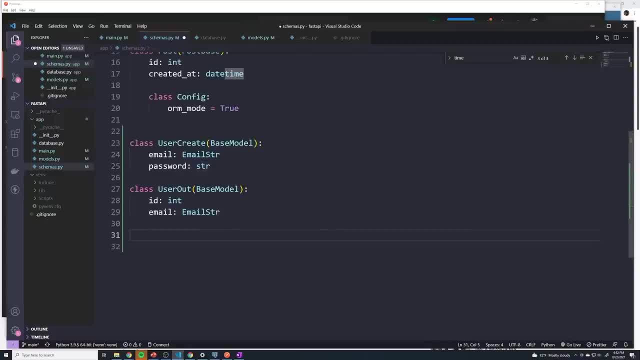 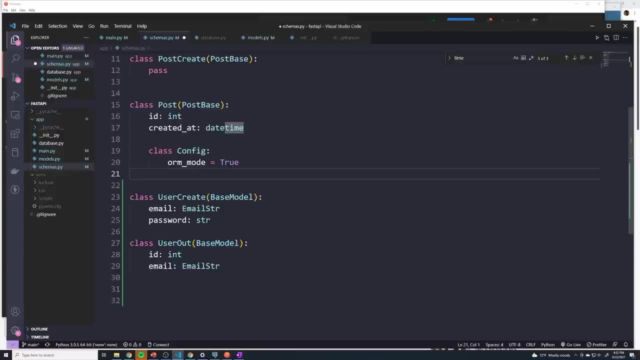 we'll just leave out password. So by leaving out password we won't ever send it back. But just like we did with the post model- remember, this is going to be a SQL alchemy model that we get and we need pydantic to convert it to a regular pydantic model. So we need this config right here. 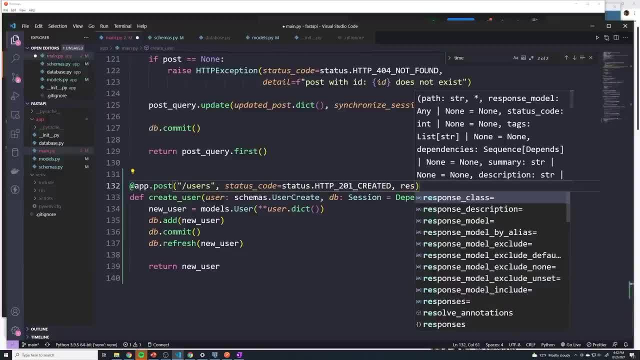 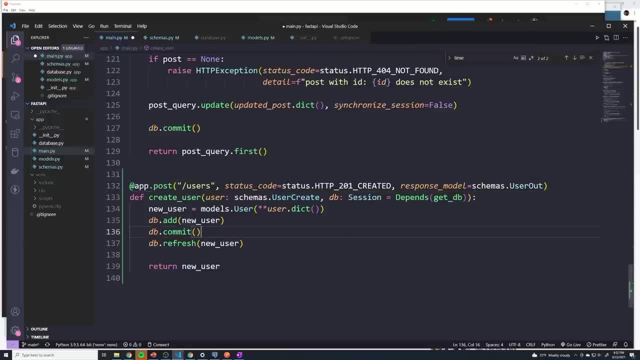 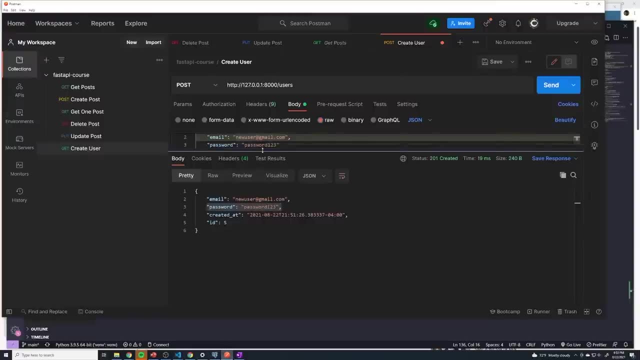 And then in our path operation we can set the response model to be schemas dot user out. All right, and then now, if I just change the fields up a little bit, create a new email. you can see that we get the ID and the email as well, But there's no password And that's. 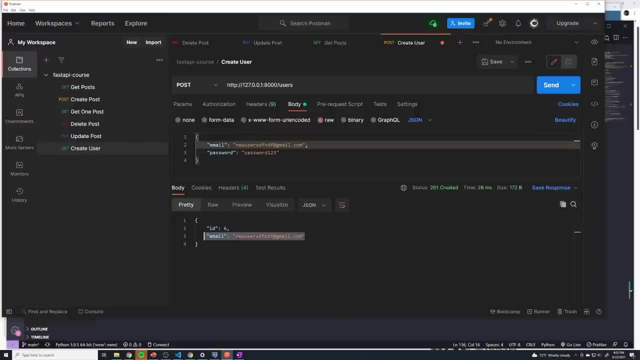 exactly what we want, And so now you guys should be fairly comfortable with being able to define a response model as well as in a request model, so that you can pick and choose whatever field you want. One last change I want to make is I want to go ahead and just add the created at field as 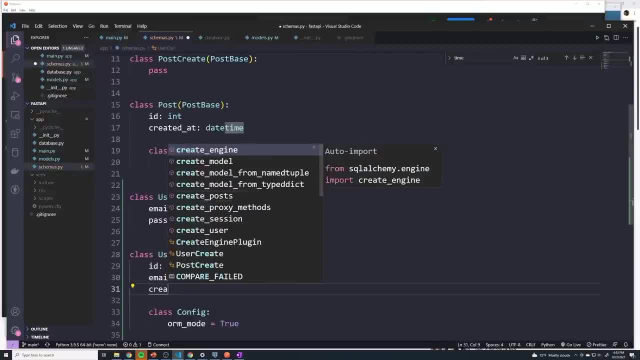 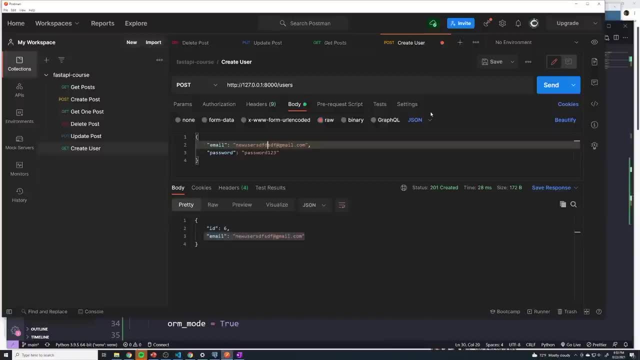 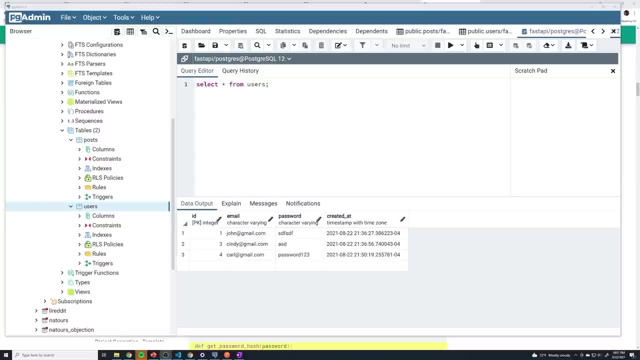 well And we can just copy this right here And so now just create another email And now we get the created field. So we got all the fields that we want. In the last lesson we handled the logic for creating a new user, But for a lot of the 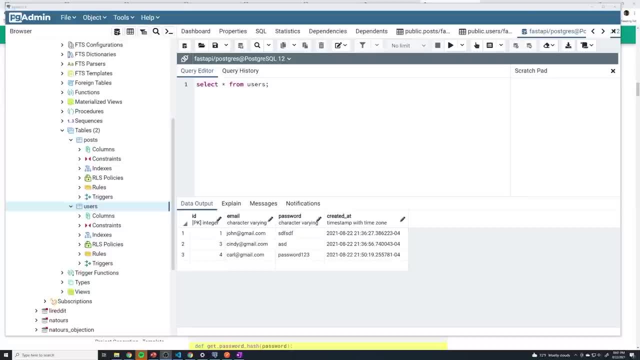 people that are familiar with security. I'm sure you guys may have had a little bit of a heart attack, Because we did something that's very, very frowned upon. we took the user's password and we just stored it as plain text within our database, And some of you might be thinking: 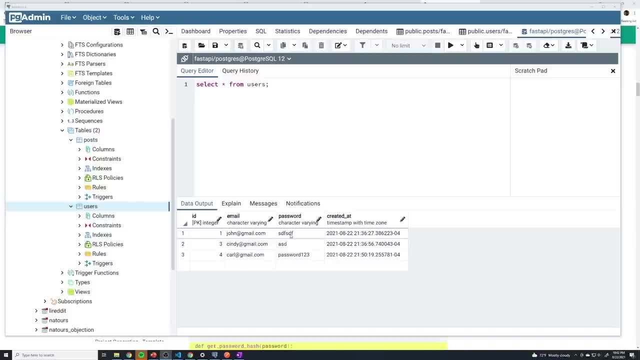 well, what's the problem with that? Right, It's in our secure database. Well, right, our database is secure for now, But there are hacks, there are things that can happen. you know these, all of these records could potentially get leaked in some. 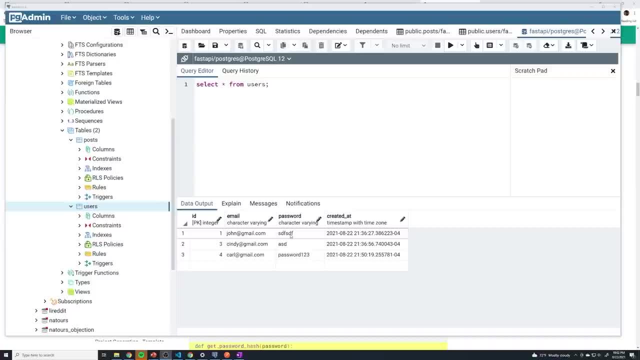 fashion And it's very dangerous to just have a user's password just stored in plain text like this that anyone can read. So when it comes to working with passwords and databases, what you always want to do is you want to hash the password. So we never store the actual password in our 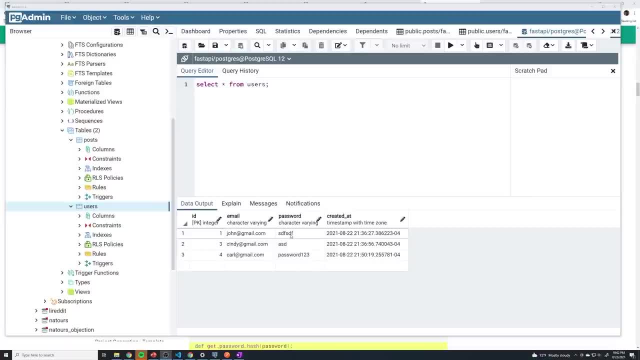 database. we just store a hash of it So that if it does get leaked, well no biggie, because it's ultimately just a hash. you can't really reverse engineer that hash and get the password. So you want to get the original password back. So in this lesson we're going to focus on hashing the 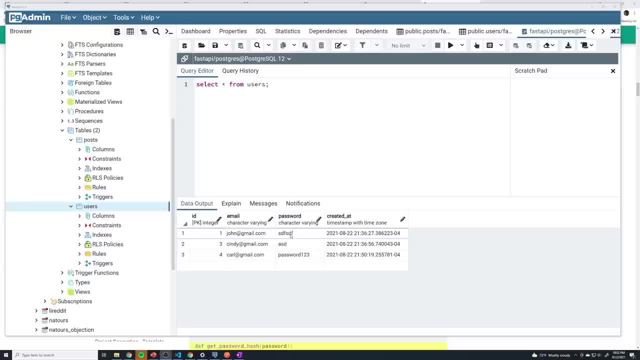 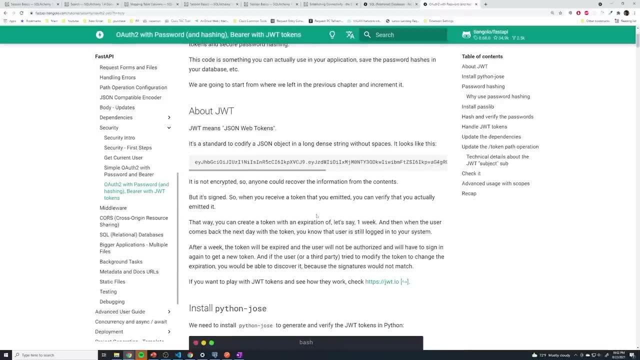 password when a user first registers, so that we never actually store the raw password within the database And within our fast API documentation. they have a good article that kind of covers how to do that. So if you go under security and then OAuth two with password, it'll show you what we 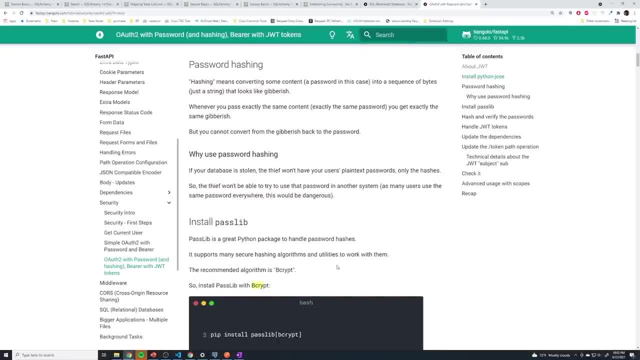 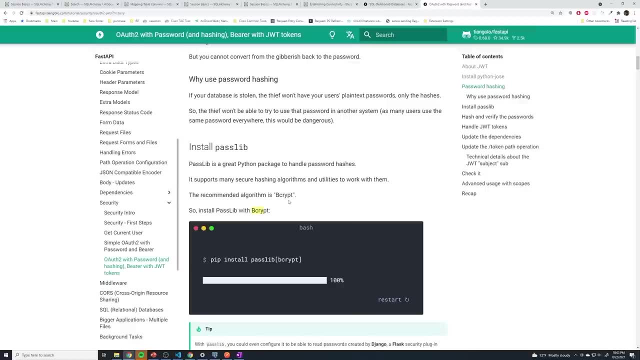 actually need to do when it comes to hashing. So there's two libraries that we need to install. Right, we need pass lib, And so that's going to kind of handle the hashing, But we need to actually specify a specific algorithm, because pass lib can work with different algorithms. One of the more popular ones is bcrypt, So we'll need 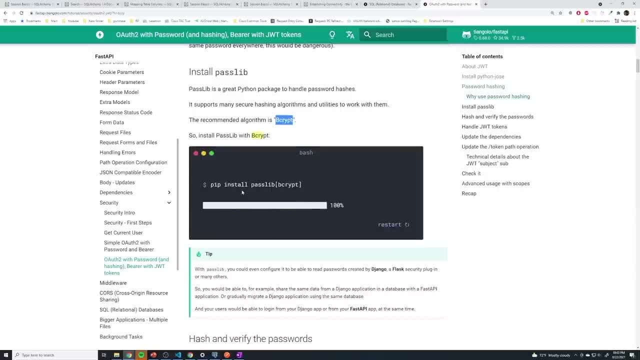 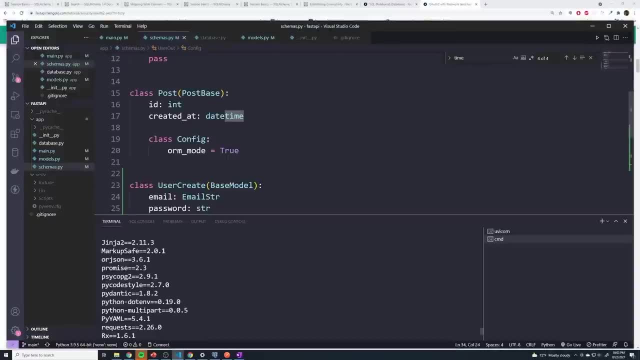 two different libraries. we'll need the pass lib and then the bcrypt library, And we can just do that by running pip: install, pass, lib, bcrypt. So I'll just copy this, We'll go to our application And I'm just going to run that command. 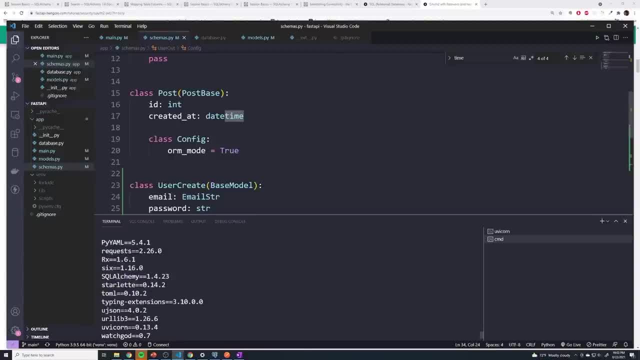 Right, and then let's just do a pip freeze just to make sure it got installed. So let's just run it. And this is the ass. So I'm going to do an install, just run it, And we can do the same thing with this. 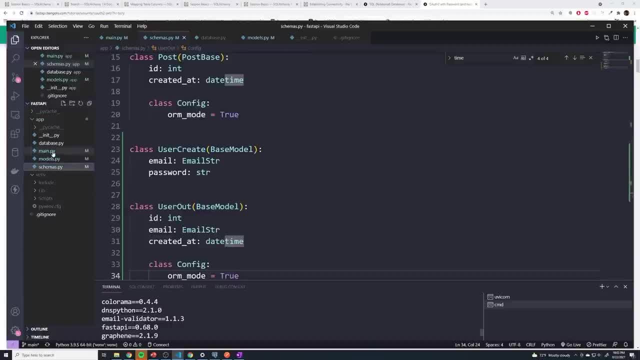 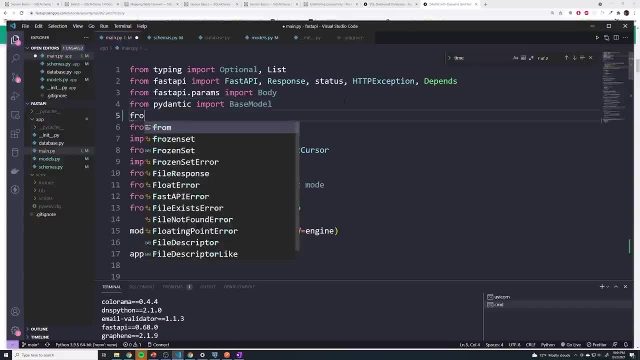 And we can just debug this, And then we see paclib there now, And then do we see bcrypt And we see bcrypt in there as well. So we've got both of the libraries that we need to actually perform the hashing. So let's go to our main file And somewhere up at the top I'm going to import from paclib dot context: import crypto context. 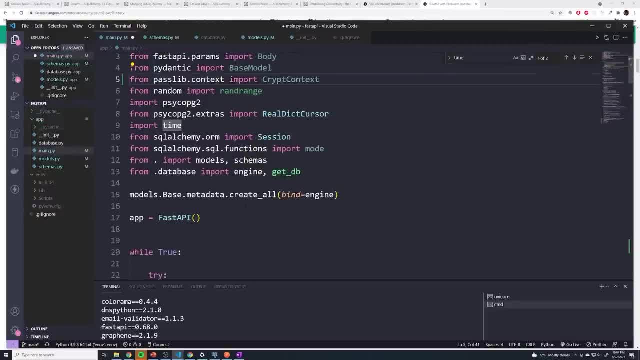 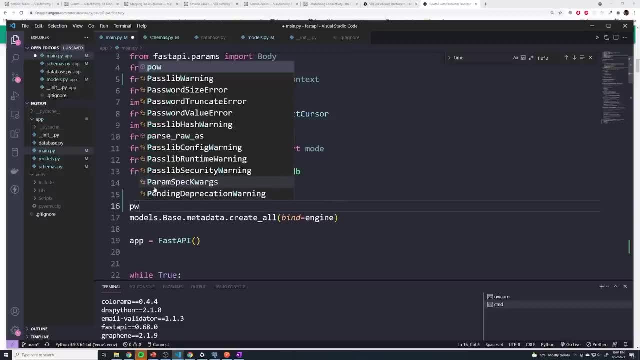 And then what we need to do is take the hash file and do an export and then import it, And then what we need to do is and place below that we have to define this setting right here, So we do pwd- underscore- context equals- and then we reference that crypto. 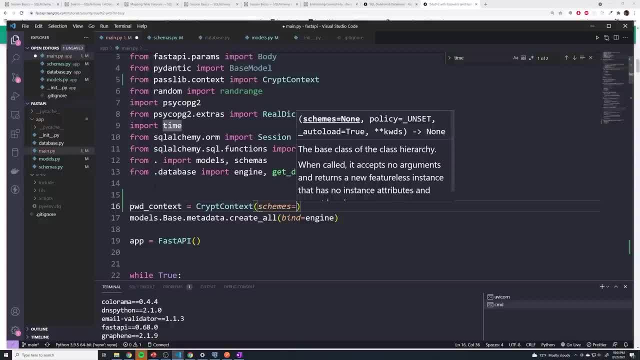 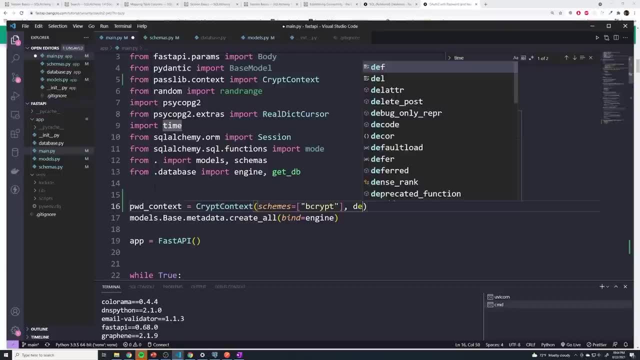 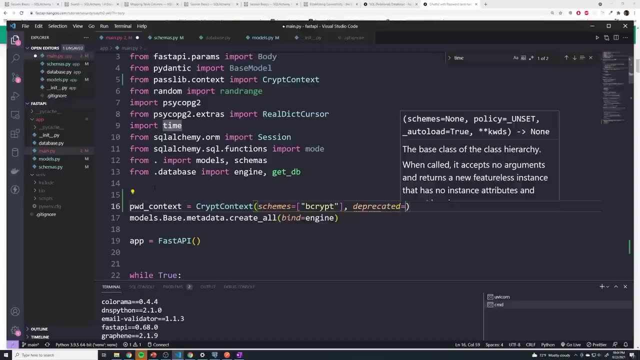 context. And then here we say: schemas equals brackets, be crypt. And then we'll do: deprecated equals auto, Alright. and so basically all we're doing is- and this is here to actually be a string- All we're doing right here is we're telling pass lib what is the default. 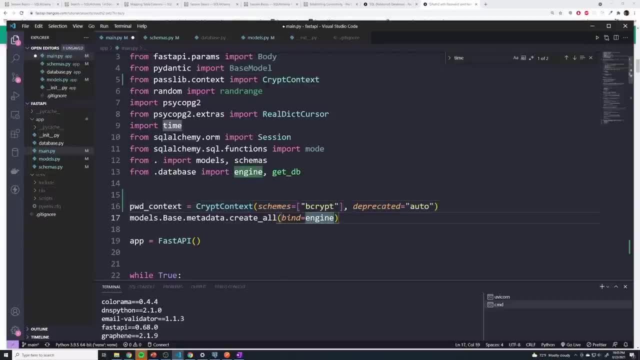 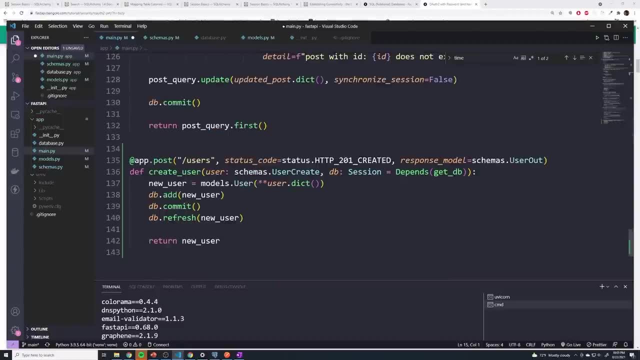 hashing algorithm, Or what hashing algorithm do we want to use? In this case, we want to use bcrypt. So that's all this is doing. Now, when we go to our user registration down here, we have to do a couple things. 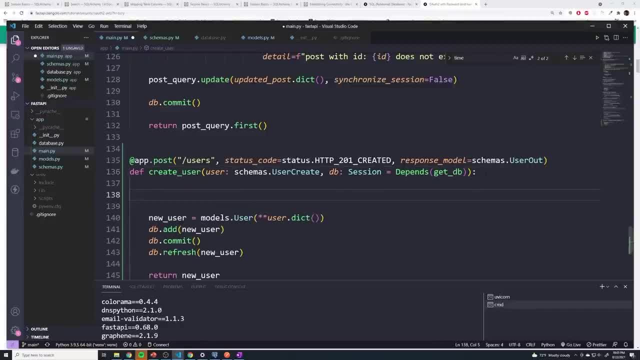 And so before we actually create the user, we need to actually create the hash of the password. So the first thing is: whoops, it's not in JavaScript land. we're going to hash the password which can be retrieved from user dot password. right, Because that's going to be stored inside. 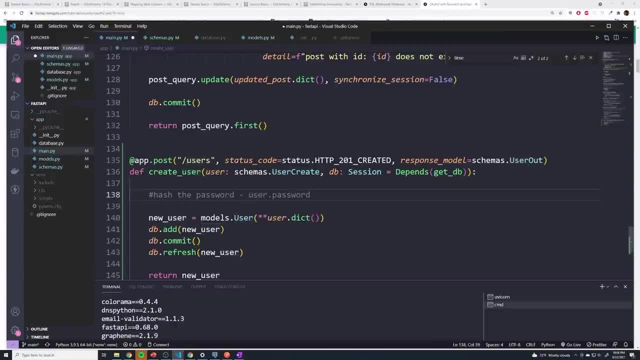 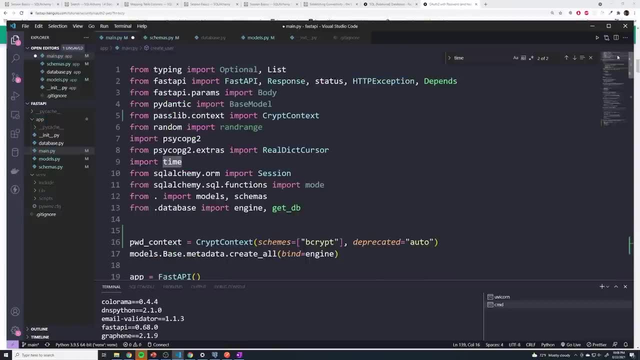 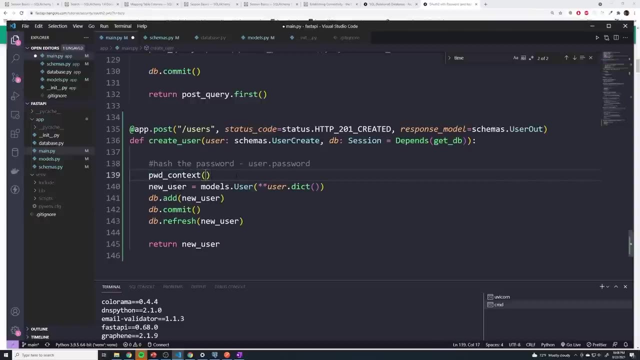 this object. And so how do we exactly do that? Well, what we can do is all we have to do is reference that password context, right? If you forgot what that is, just go all the way up to the top. That's this command right here. So we reference password context And we call the hash method. 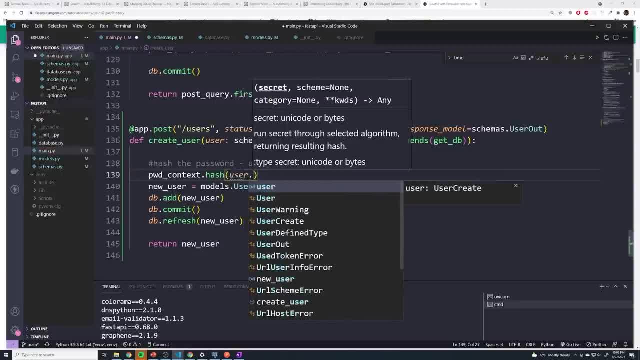 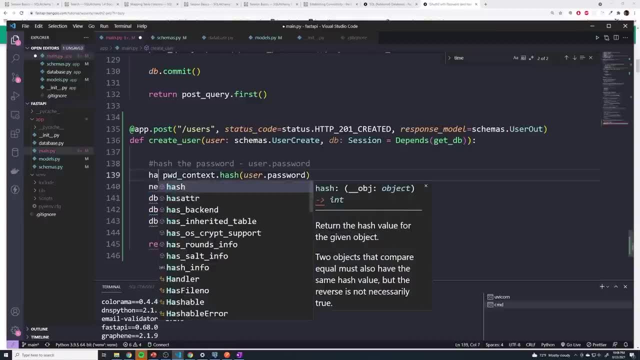 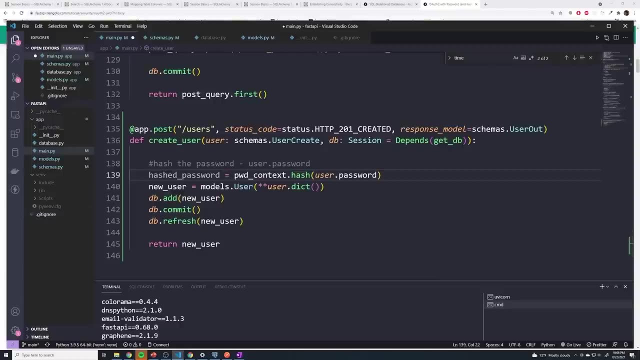 So that's going to perform a hash, and then we just pass in user dot password And then we can store this in a variable called hashed underscore password, And then what we're going to do here is we're going to take the user dot password. 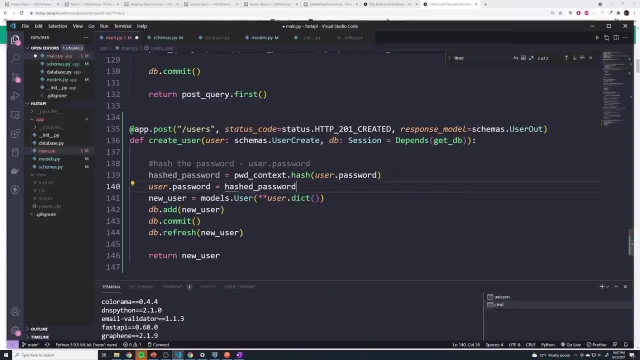 And we're going to set that now to the new hashed password That's going to update the pydantic user model, And then at that point we can just leave everything as is right. So we hash the password. so we got a hash and then we stored it under user password. 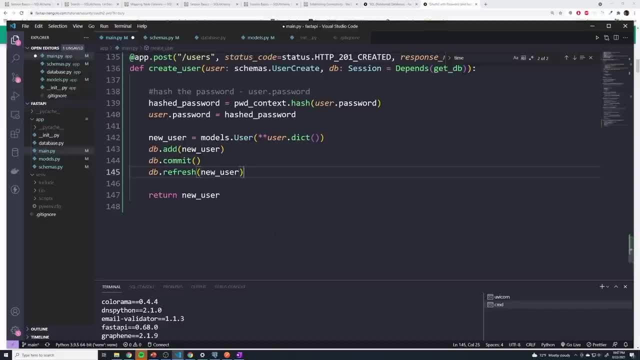 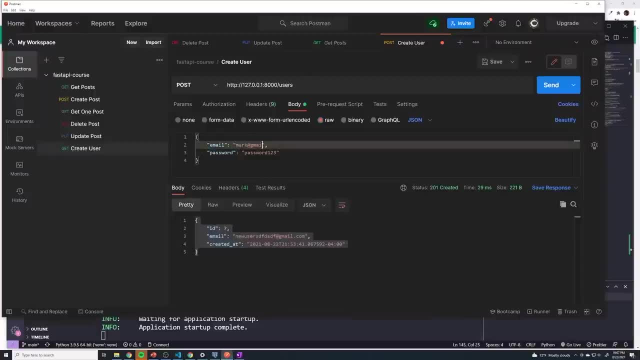 and then everything else can just be kept the same. So let's actually try this out And let me just double check to see there's no errors- and there isn't. So let's create a brand new user And I'll call this mark at gmailcom: Same password. that's fine. 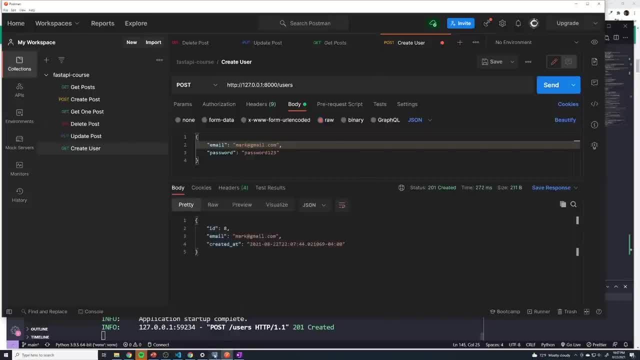 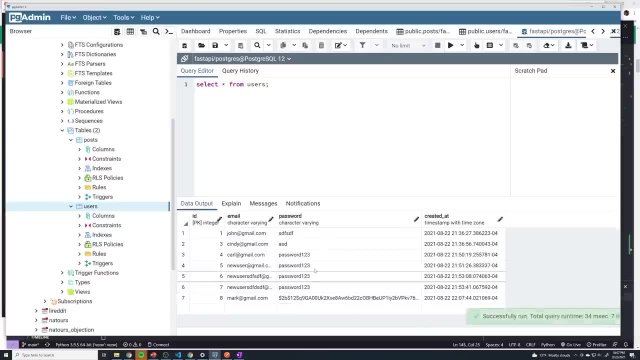 Okay, Send, it looks like everything worked, And then let's just run this, And then, if you see that most recent user, you can see that we no longer store the raw password, we store a hash of it, And so that's going to help it be a little bit more secure. Because if 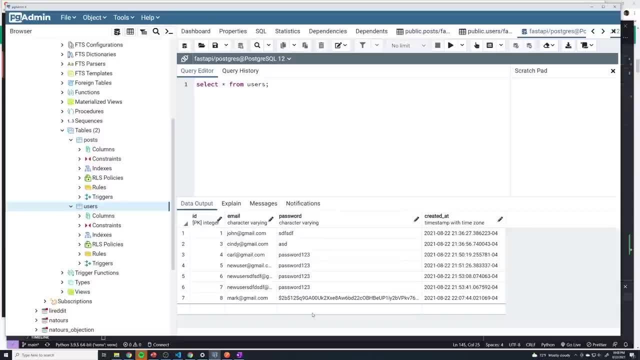 it does leak, then you know the hackers will only get access to a hashed password and they can't exactly convert it back to the original password. That's the great part about hashing. It's a one way street. we hash it, we only get the final password. you can never. 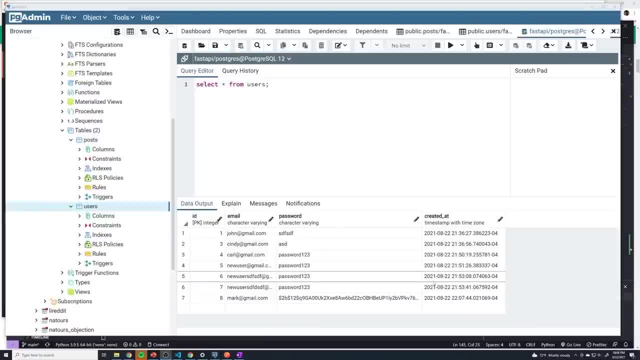 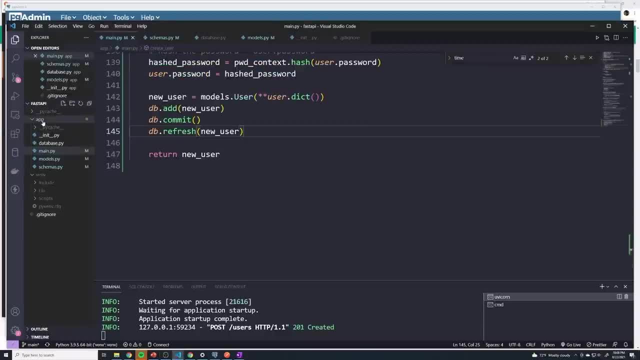 put it back into a function to convert it back to a password. Now one thing I want to do is I want to extract all of the hashing logic and store it in its own function. So I'm going to create a new file And I call. 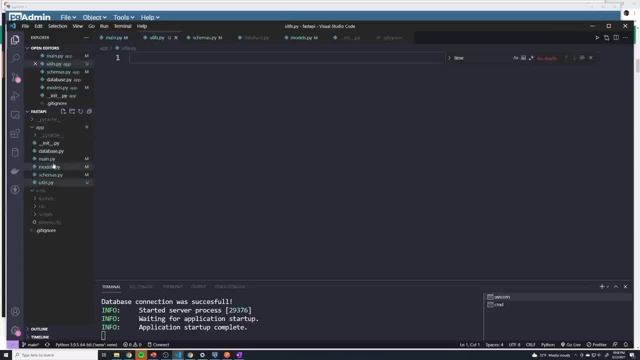 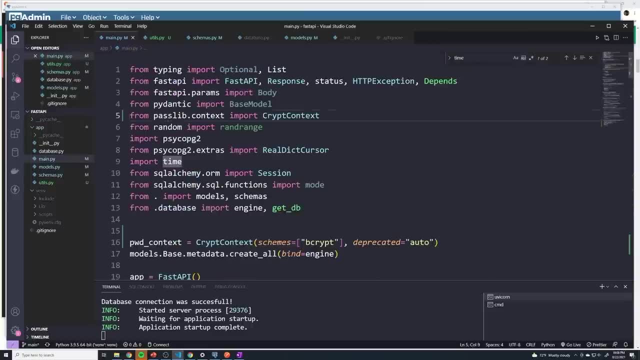 this: utils dot p, y, These are: this file is just going to hold a bunch of utility functions, And what I'm going to do is I'm going to go to our main file And I'm going to remove this line, or cut it, And we're going to paste it into my utils file, And then we're also. 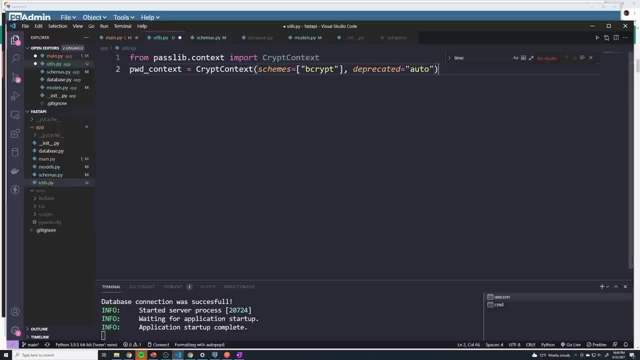 going to cut this out. Okay, move all of this logic into here, And then we're going to define a function that we can call, and I'm going to call this function hash, And it's going to take a password, which is going to be of type string, And all it's going to do is it's going to return pwd context. 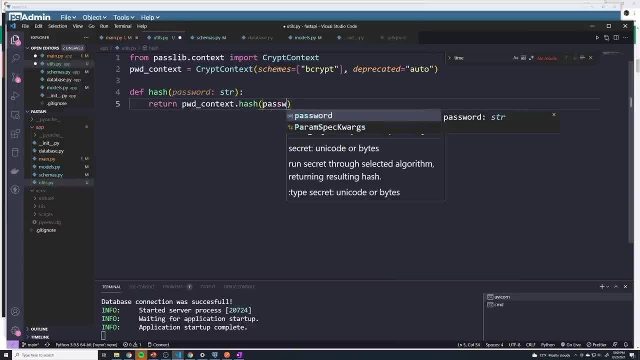 dot hash of whatever the password the user passes in, And that way we really extract and place all of the hashing logic into one file or one function, So we don't have to import all of this nonsense into other files And then in our main dot. 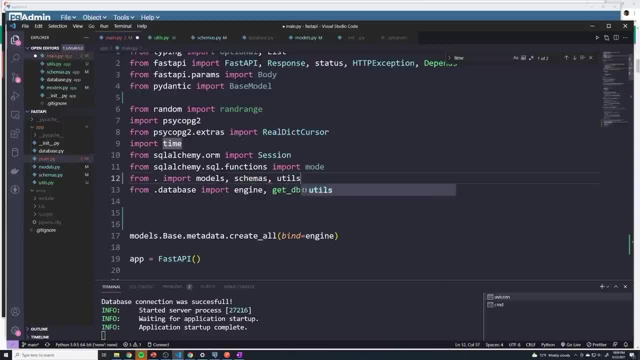 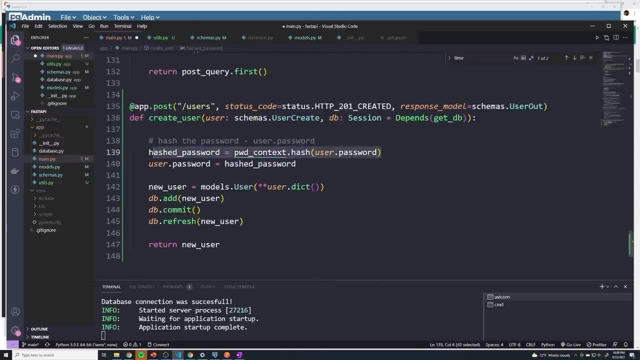 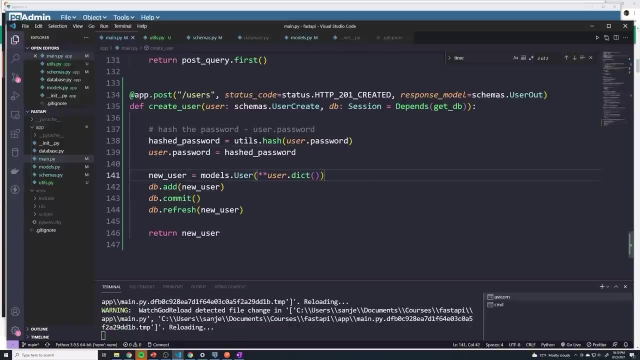 p y file. we can import utils And then down here what we can do is, instead of calling this, I can just call utils dot hash, And then we'll pass in the user password again, And this shouldn't really change anything else in our boat. 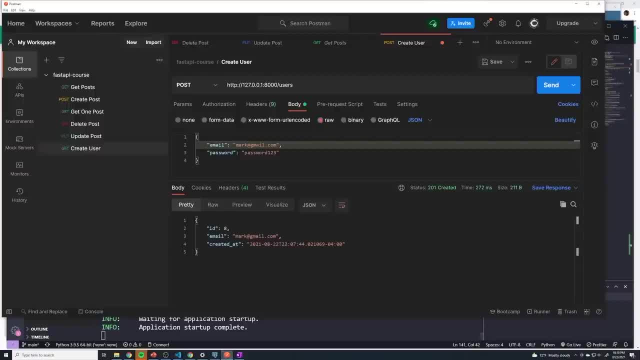 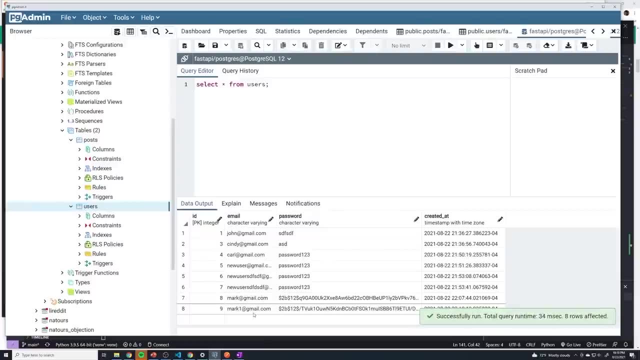 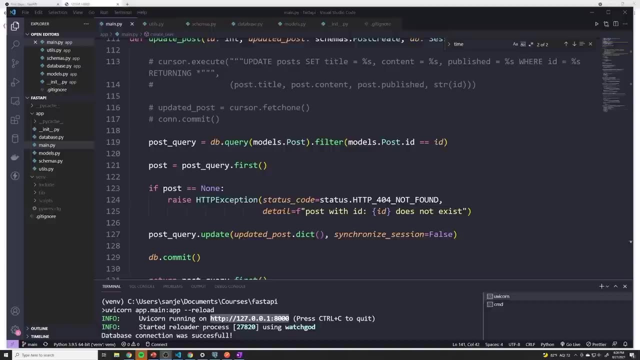 code. Let's try this again. I'll create a. I'll just add a one here. Then seems to work. Let's just double check. And the second user, the password was properly hashed. The next thing I want to do is I want to set up a route or a path operation that allows you to fetch. 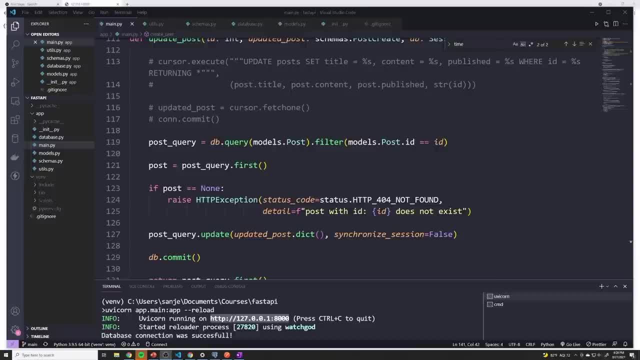 and retrieve information about a user based off of their ID, And there's a couple of different reasons why I want to do this. One of them is it can be part of the authentication process. So, depending on how you set up the front end, if you decide to, you know, set up JWT. 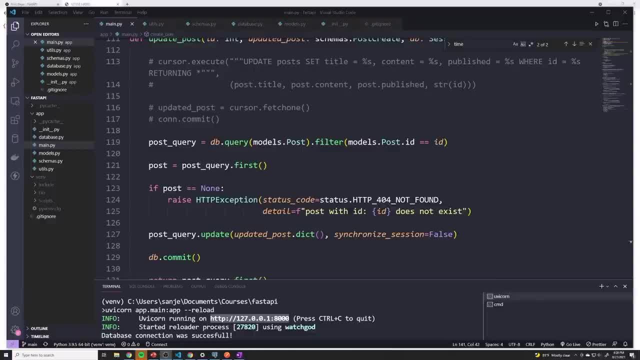 tokens to get sent as cookies, then the front end may not actually know whether it's logged in or not, And so a lot of times you'll see some API's have an endpoint to let you kind of retrieve information about your own account, And so if you're able to access it, that means 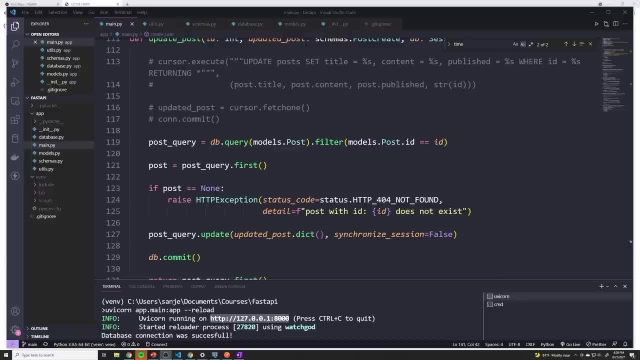 you're logged in. If you're not, then you know that you need to fetch a new token. Also, there's other reasons why you want to do this too. 00.07. You know if you're working with other API. you know if you're working with an other API, you know. 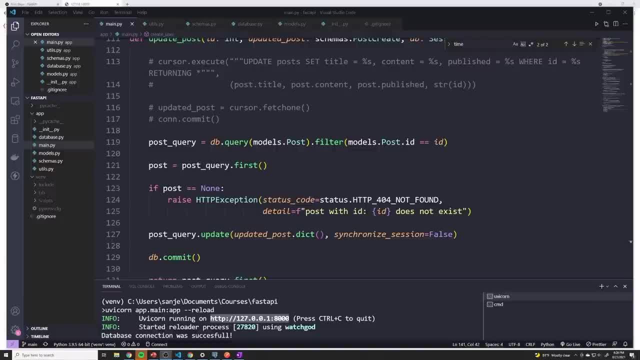 you're, you know, thinking taking a look at something like Twitter: right, you need to retrieve a user's profile if you want to view it, And so in your API, you're going to have to set up a route so that people can retrieve someone's profile information, And so that's why I want to 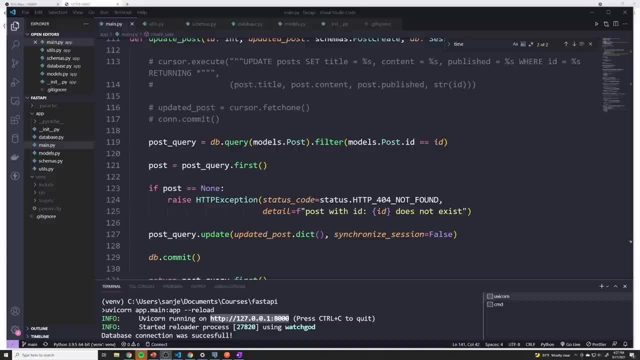 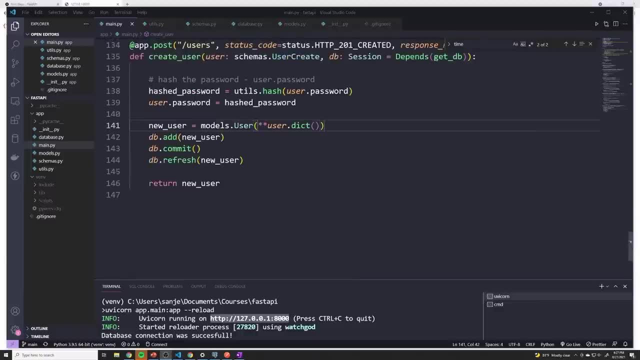 set up this route. I haven't really decided what we're going to ultimately do with it, But for now I just want to set it up so that you can retrieve information about a specific user based off of their ID. Let's go to the bottom of our code here And we'll create a new path operation. 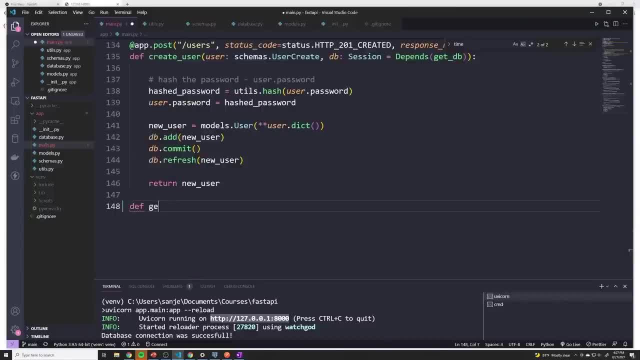 And I'll call this. I get user And before we do that I'm also going to set up the decorator. So this is going to be a get operation, because we're going to treat the information about a specific user And the specific path is going to be slash users and then slash ID, So kind of like how we 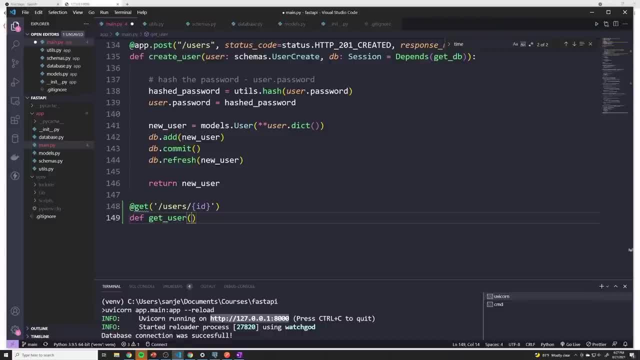 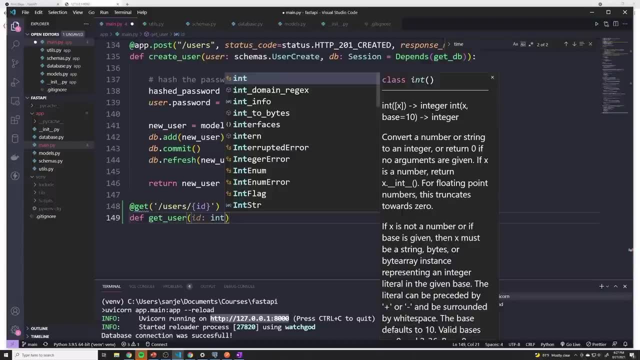 did when it comes to retrieving a specific post. we're going to pass in the ID in the URL, And then we have to extract the ID from the URL, And then we have to extract the ID from the URL, And then I'm going to make sure that we validate it as an integer, And the next thing that we have to do is 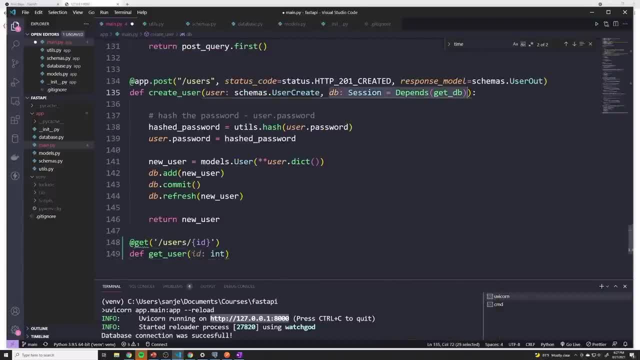 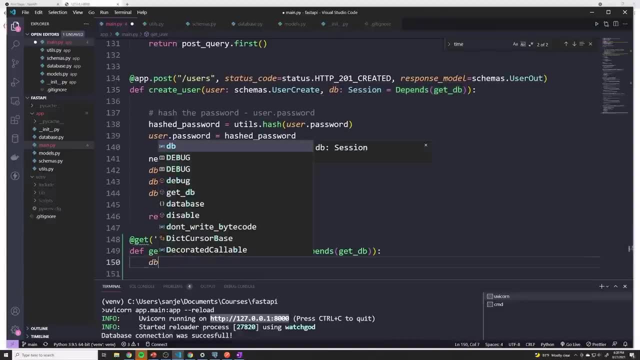 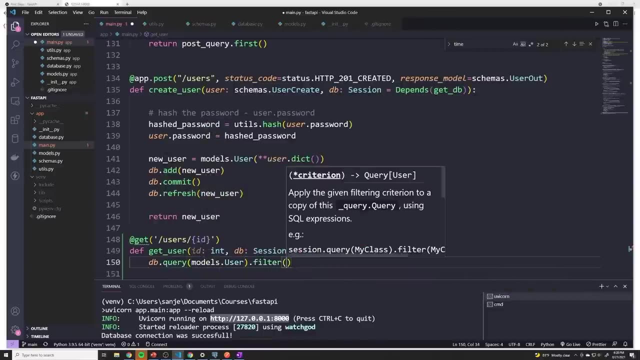 since we're going to be interacting with the database, we need our DB right here. So we'll copy that And then in our actual function we're going to do a quick query. So we'll do DB dot query And then we'll grab models, dot, user And I'll say I want to filter and then look for. 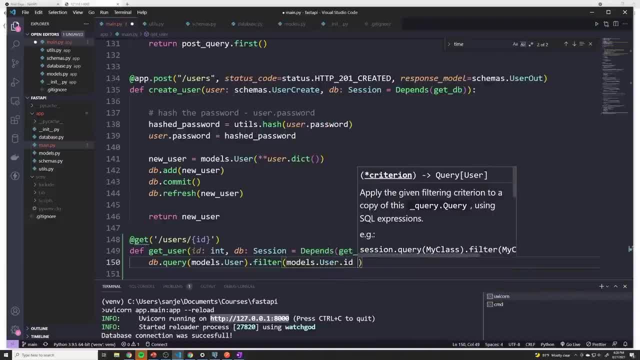 something with models, dot, user, dot, ID equals, equals and then it's going to match up with the ID that they've requested And because there should only be one user with a specific ID, we're going to just grab the first one, So we don't spend extra resources looking through the rest of our database. 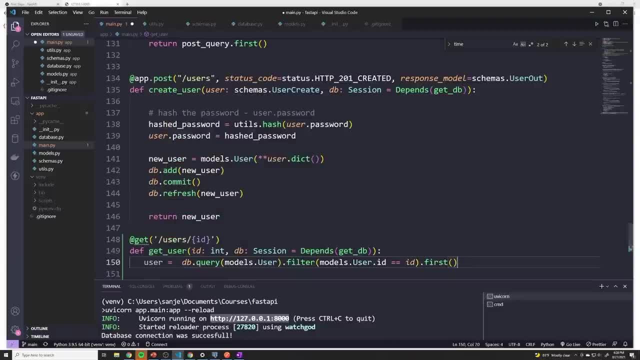 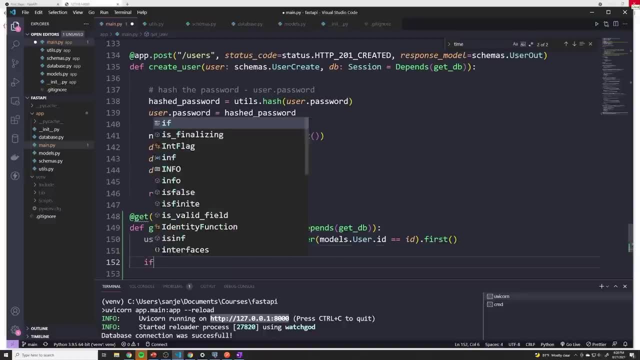 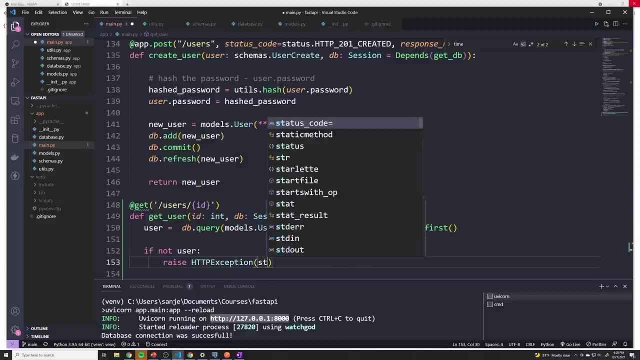 And we're going to store this in a variable called user. All right, and then, just like we did for fetching a specific post, if a user was not found, so if not user, we'll say we want to raise an HTTP exception And we'll say the status code equals. 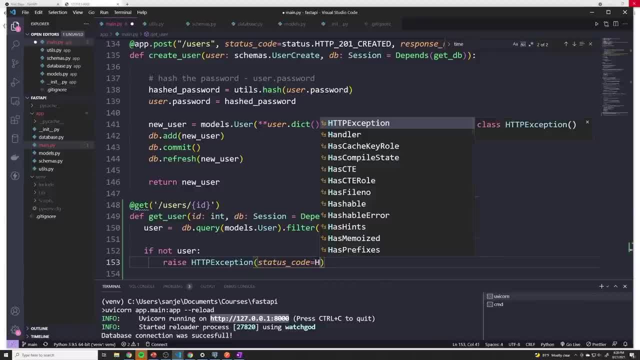 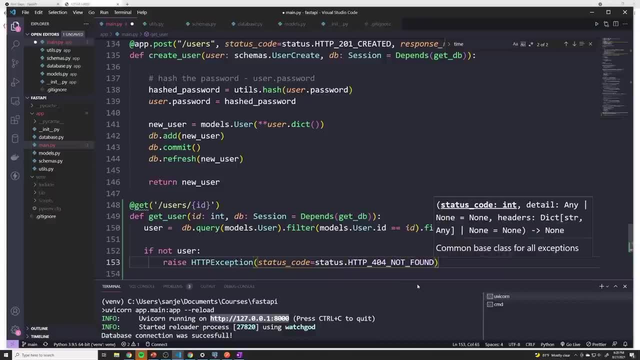 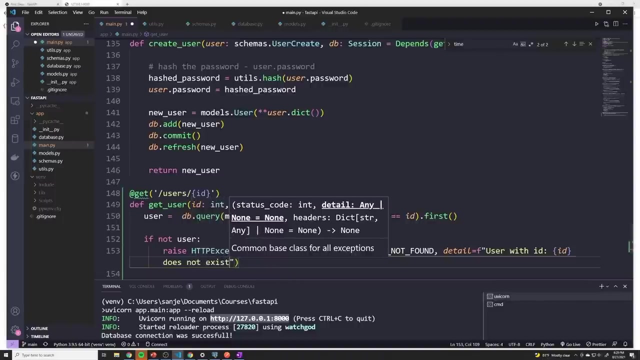 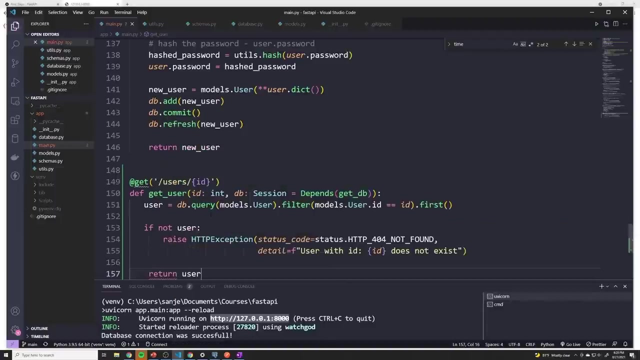 404, whoops, HTTP status dot, and then we'll grab 404.. And the detail is going to be: user with ID and we'll pass in. the ID does not exist, But if the user is properly found, we will return the user And it looks like there's some kind of 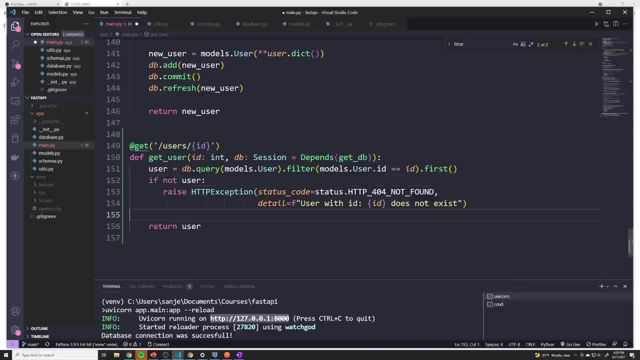 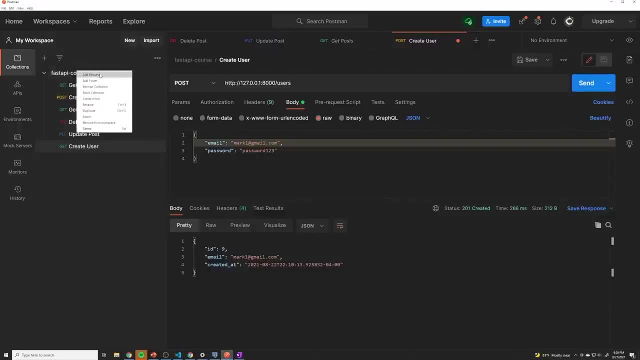 weird issue with my formatting. So, all right, there we go, And so let's just quickly test this out. So, once again, I'm going to create a new request And we're going to make sure to save this one, And I'm gonna call this a get user Copy this URL. it's going to be the same same route as just. 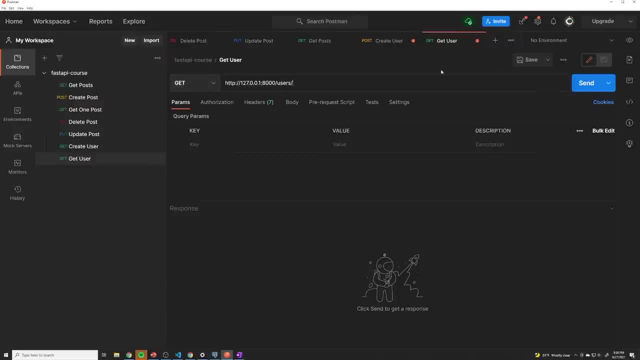 it's just gonna be a get operation And then we want to send a specific ID. So I take a look at your database and then see if you can grab an ID that does exist. So let's just say one, we'll hit send And it looks like there's some kind of issue because I'm not getting a response. 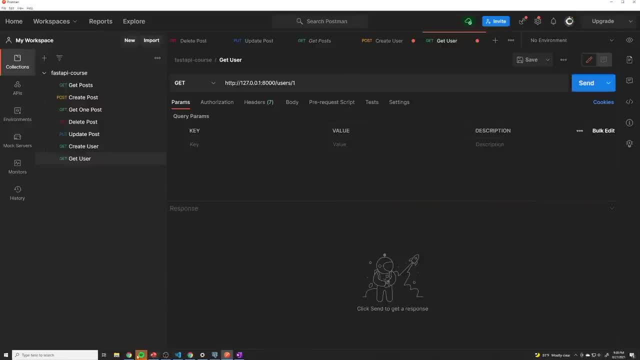 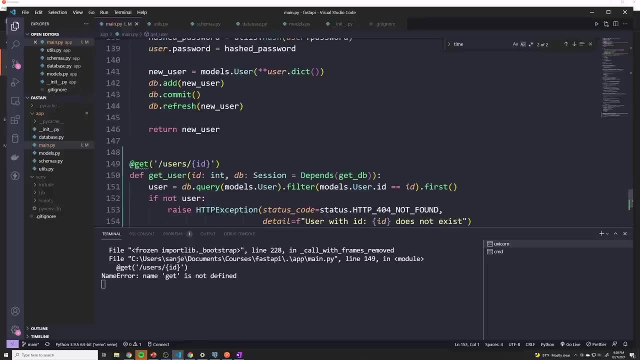 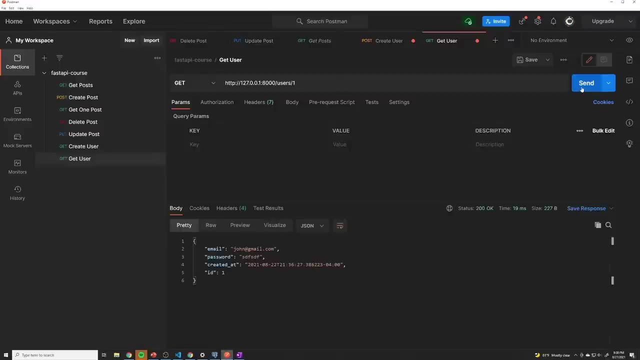 yet. But let me cancel out of that And let's see what we did wrong. And I realized I forgot to do app dot get Great. so we actually got the user. everything seems to be working. However, there's one little issue. First of all, we should not be getting the password right. We never want. 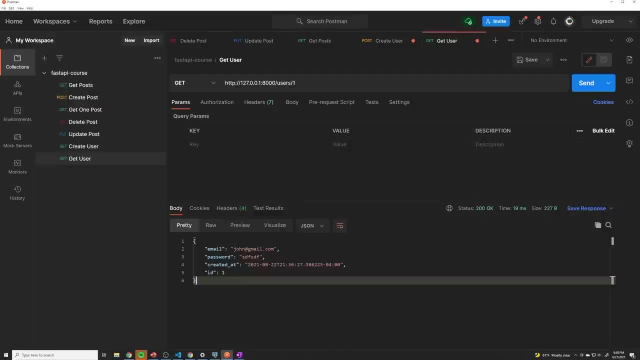 to return the password to the user. the user already knows his password. And also, if you want to, if this route is so that you can retrieve a user's profile, kind of like you can on Twitter, Instagram, then we're sharing someone else's password And that's a little bit of an issue. 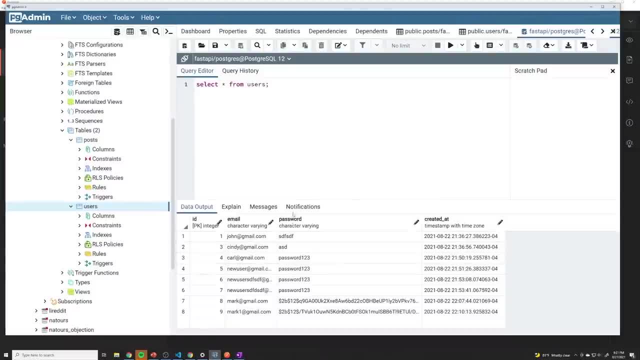 And the reason why this isn't a hash password was because I didn't clear out my database before we implemented the the hashing of the password. So that's why it's in clear text. But whether it's hashed or not, you never want to send this out, right? You don't want anyone. 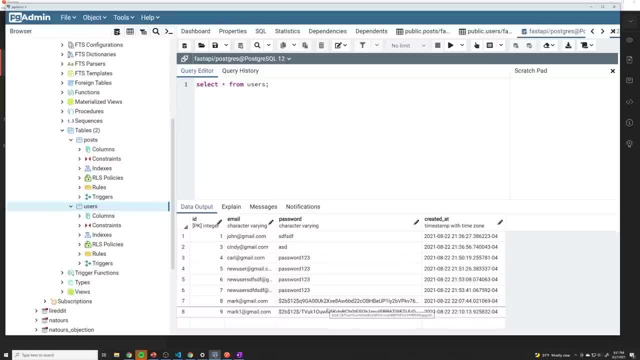 else to see your password. you don't even want the user to see their own password, because someone else could intercept it and potentially do malicious activity with that information. So what we're going to do is we're going to filter out that specific field, just. 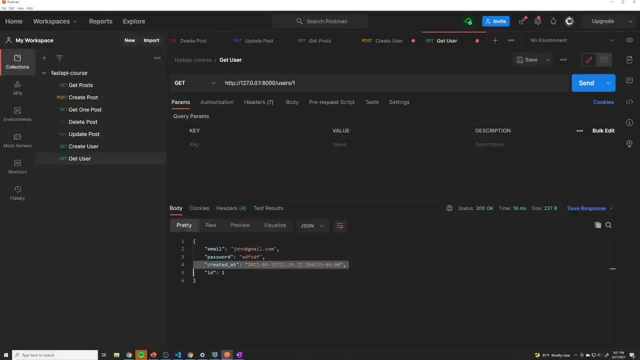 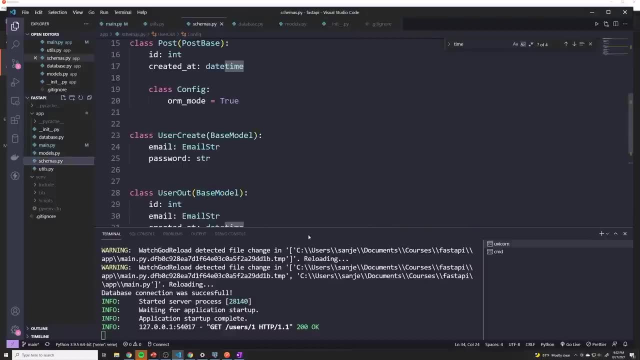 the password field. I want them to be able to get the ID to create that field and the email Speaker 1 and any other fields outside of the password. And fortunately for us, if we go to our schemas, we've actually already defined a schema for the user out. So this is: 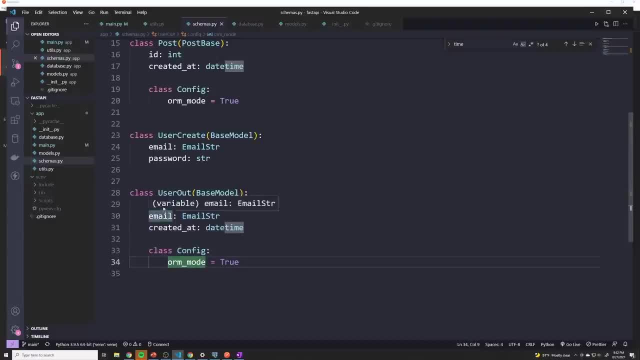 going to be any information about the specific user, except we're extracting out the specific password And so we can just set the response model to be user out And we'll go back to mainpy and we'll say response dot model. And we'll go back to mainpy and we'll say response dot model. 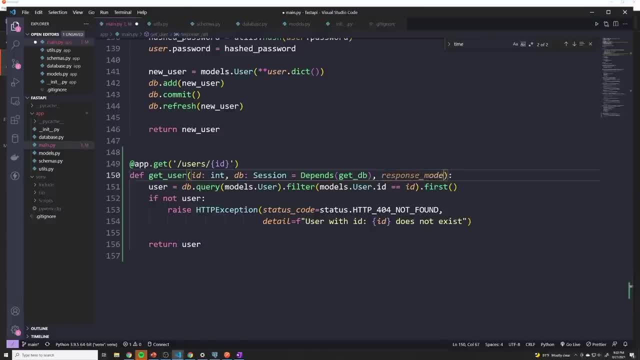 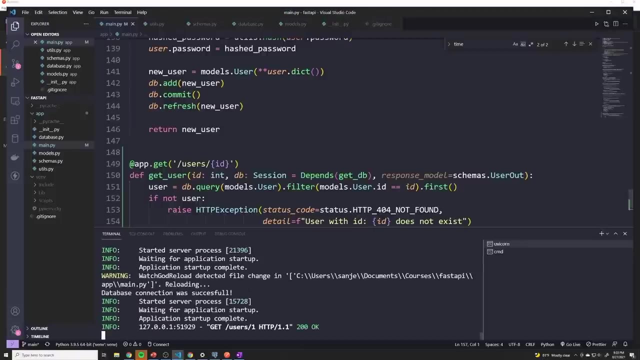 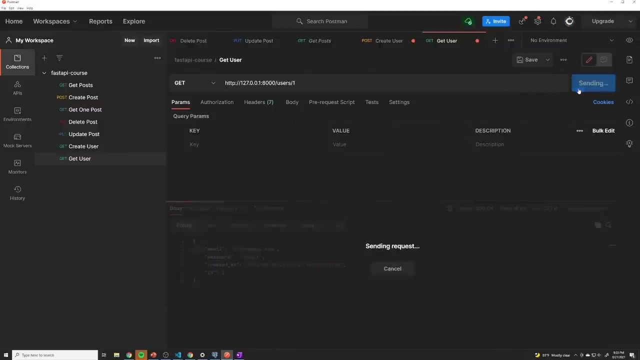 Sorry, response. underscore. model equals schemas. dot user out. All right, we'll save this And we'll try this again. So we'll retrieve this user And we still got the password. So what happened here? And this could just be an issue of me not saving, So let's try this again. Still a little bit of an. 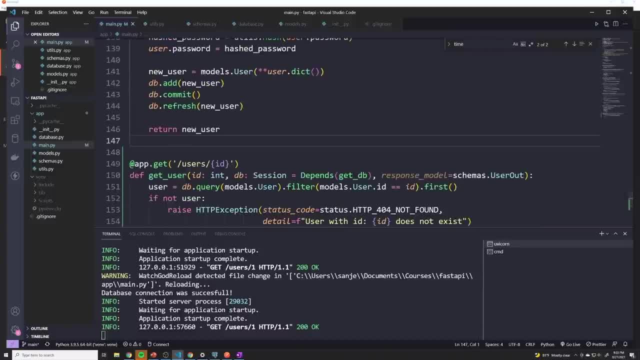 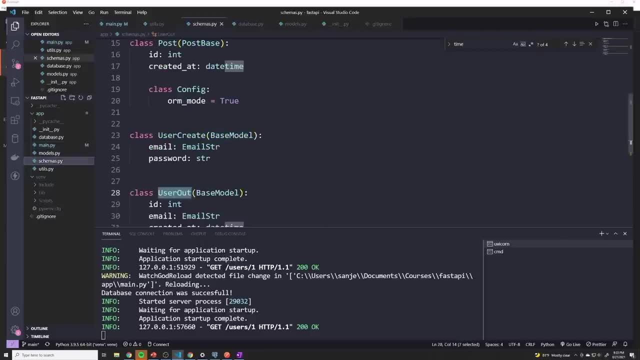 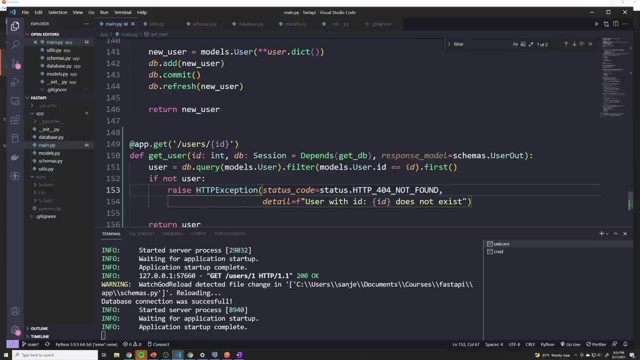 issue And let's just make sure I imported schemas. I did, And let's go to our schemas, And I've said just these fields, So this should be good to go. I'm not sure why it's giving us errors And I made a stupid mistake. This should not be. 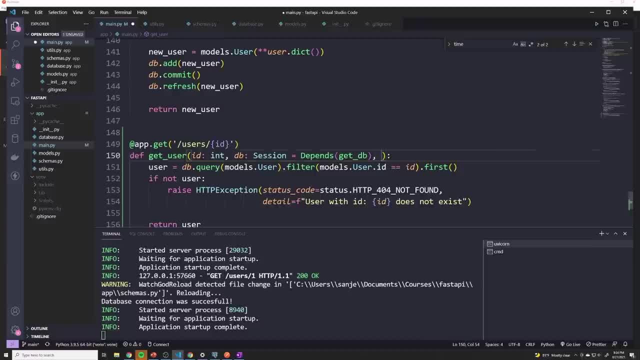 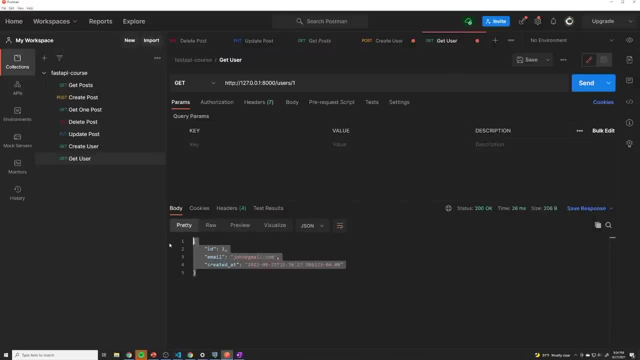 within the function parameters. This should actually go inside the decorator. So it wasn't actually doing anything. And now, if we try this, we can see that the password field has been successfully removed, Now that we've added a couple of path operations for users, if you take. 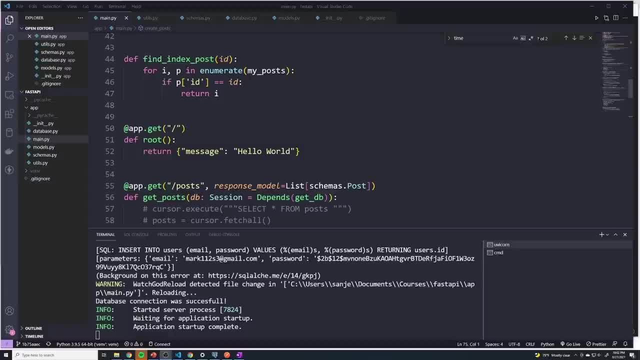 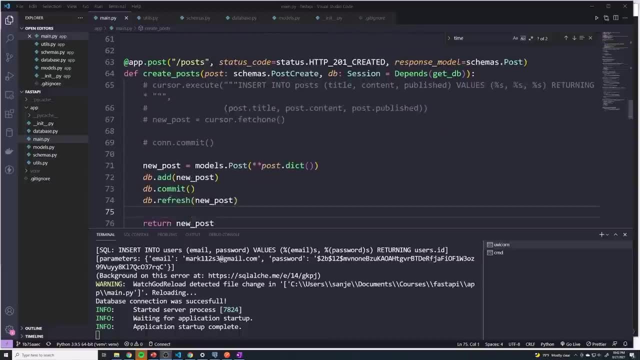 a look at our mainpy file. it's starting to look a little cluttered And you'll see that we've got all of our path operations for, you know, handling CRUD operations for posts, And then you'll see that we also have all of our path operations for working with users. So that's creating users. 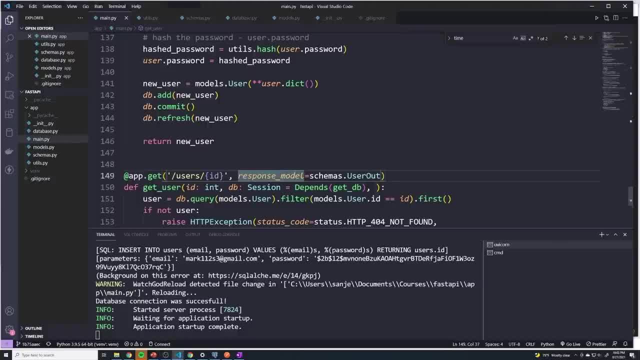 as well as retrieving a user by ID. And you know, as I said, this is a little messy And as we keep adding more and more path operations, it just seems almost impossible to keep up with that. So that's seems almost unmanageable to keep everything in a mainpy file, And instead what I want to do is 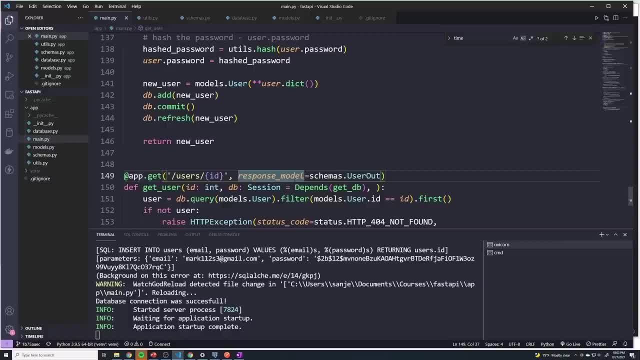 I want to break it out And I want to create two separate files, And one file is going to be for all of the routes or path operations that work and deal with posts, And then I want a separate file that will handle all of the path operations for working with users, And you know it's not. 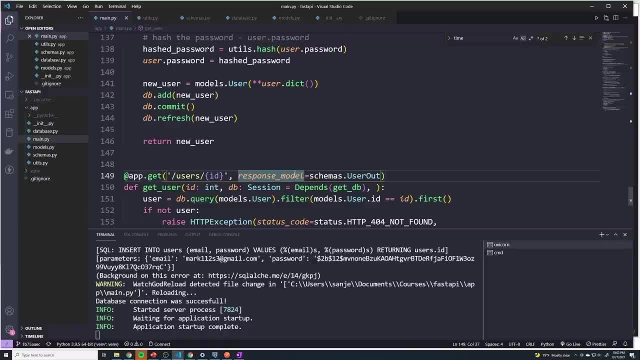 quite as simple as just, you know, moving these path operations to different files. we do have to learn about something specific to fast API, And this is nothing unique about fast API. you'll see that every single web framework is going to have a way to kind of accomplish this, And it. 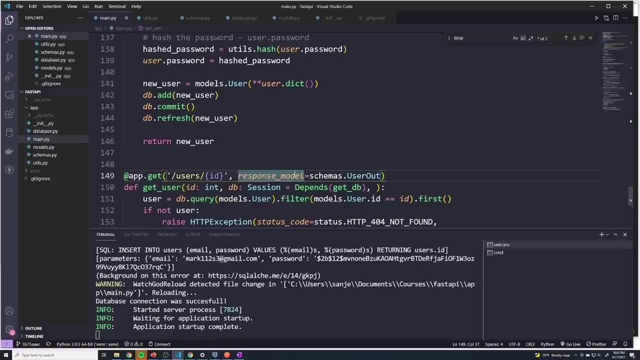 usually involves something called routers. So we'll take a look at routers in this section and how we can use them to actually split up all of our path operations so that we can organize our code a little bit better. And so what we're going to do is we're going to create a new folder. 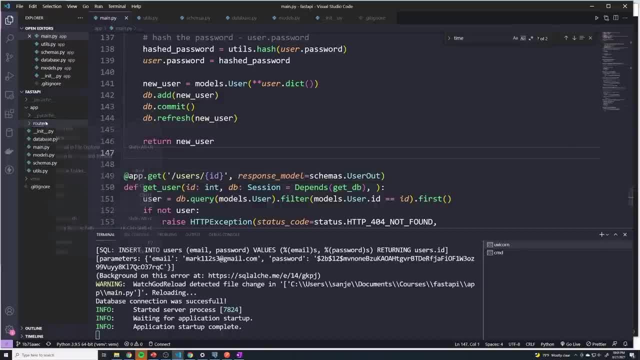 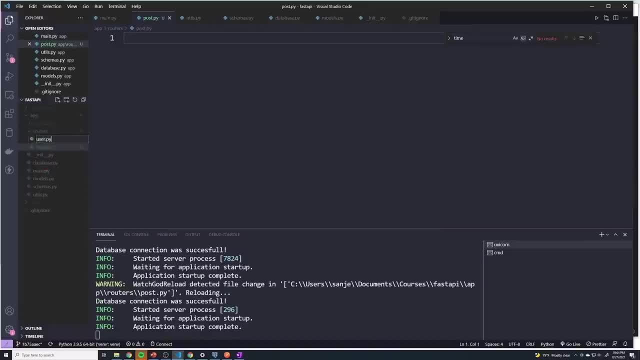 And I'm going to call this routers. And then within here I'm going to create two files. I'm going to create one called postpy And I'm going to create one that's called userpy. So all of our path operations dealing with users is going to be put into this file And all of our path. 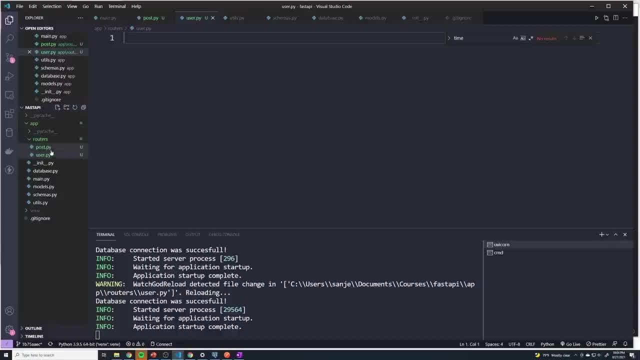 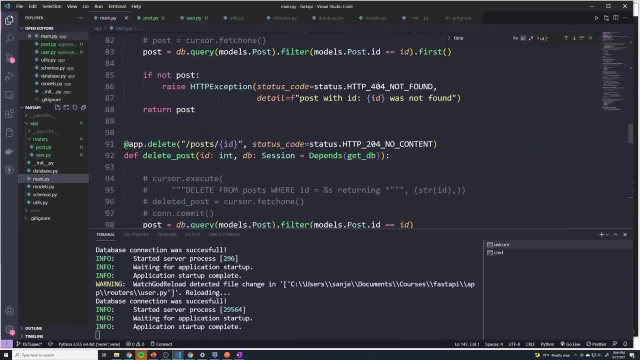 operations dealing with posts is going to be put into this file, And what I'm going to do is we're going to go to our mainpy file And I'm actually just going to copy all of my specific routes that deal with posts. first, 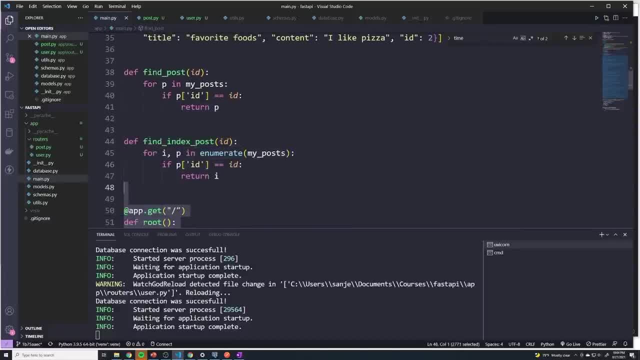 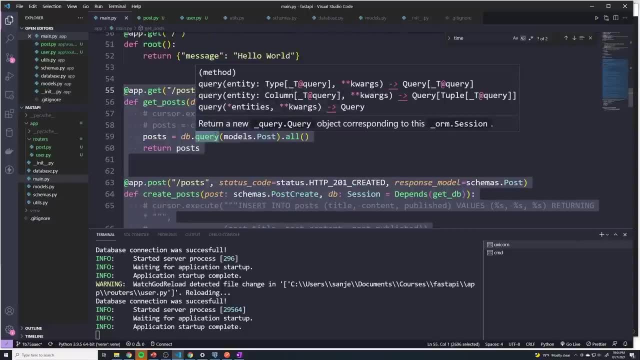 So we're just going to keep going up, and I went too far up. Oh, this thing moves quickly. Here we go. This is going to grab all of our posts And I'm going to just cut that out And we're just. 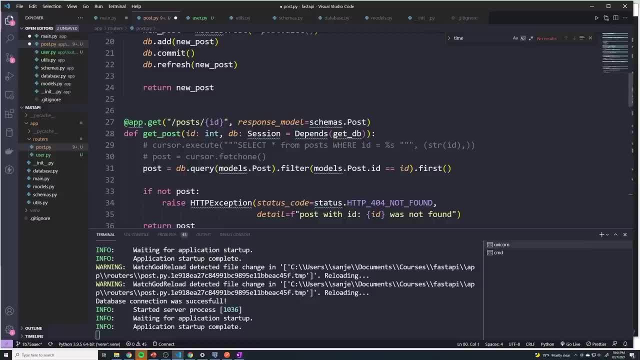 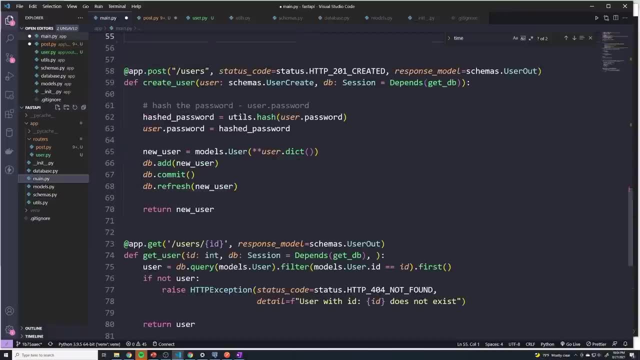 paste it in here And there should be plenty of warnings and errors within VS code. That's to be expected. Don't worry about that. We'll fix that in a bit. I'm going to do the same thing for the users. So let's go to our mainpy file and just grab the last two path operations that we have. 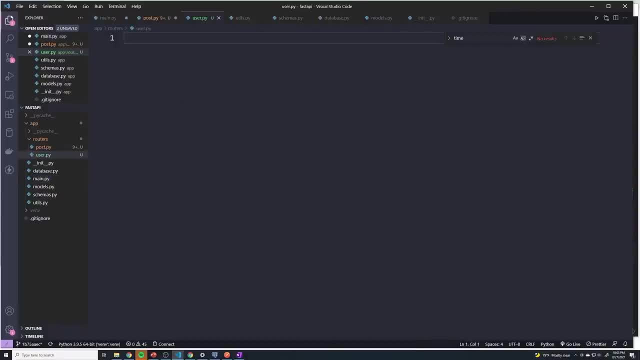 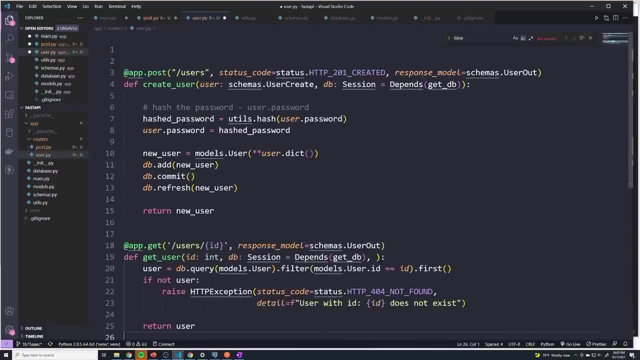 for users And then paste it into this specific file, Right? so we've got a bunch of errors And let's go ahead and actually fix those first, before we actually start working with routers. And so now that all of the the path operations are within these files, we're going to have to import. you know things. 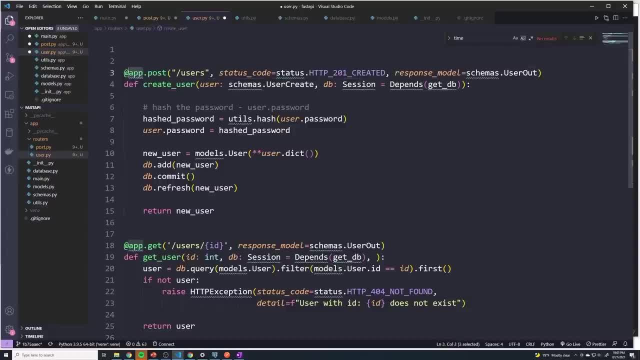 like app we're going to have to import. well, we'll come back to that. actually, we'll have to import status. we'll have to import our schemas. we'll have to import the session object. we'll have to import all of our database related things. 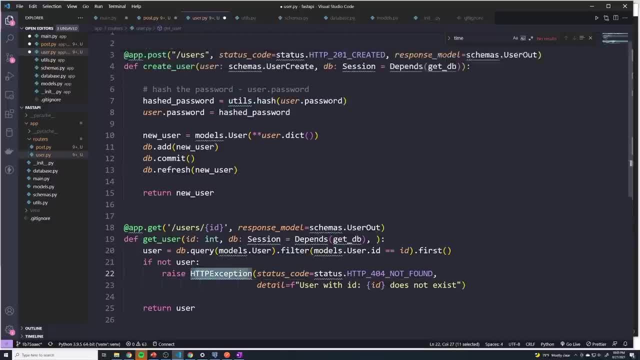 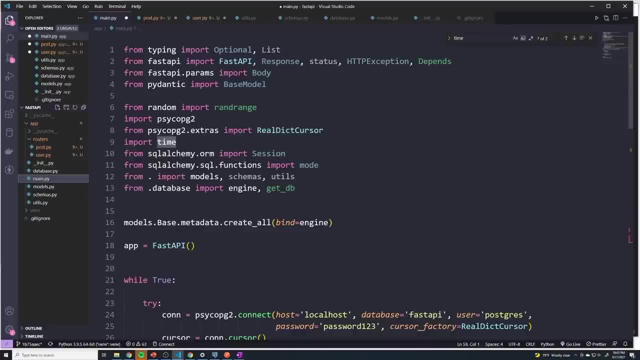 utils. So all of these things that we see little squiggly lines, we have to import them because we had already imported all of these in the mainpy file, And so we'll start off by importing the models, the schemas and the utils folder. if we need it for one of the specific files you'll see. 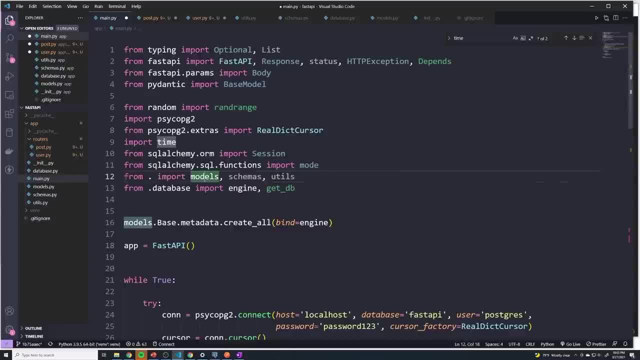 that we only need this for the user file, And so the way we did it in our mainpy file is we say from, and then this dot means current directory, So we say hey, from this current directory we're in, which is- if I kind of close that out, you can see that everything is in the app file, app folder. 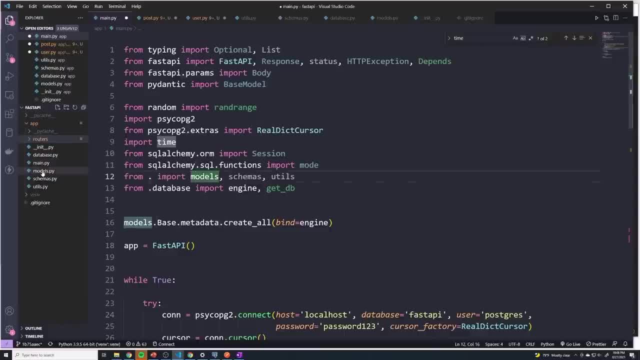 sorry, we're saying from the current app directory I want to import models, which is right here, And I want to import schemas and utils. However, in our userpy file, in our postpy file, the models, schemas and utils folder is not in the same directory because we actually have to go up a 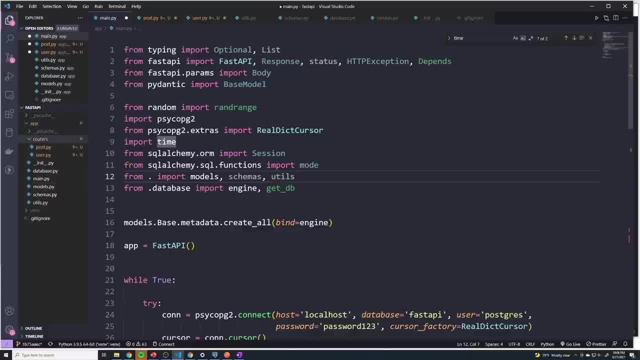 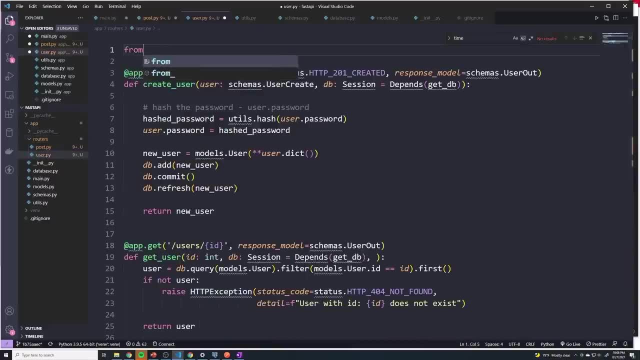 directory to the app folder to access them. So instead of doing one dot if you want to go up a directory, you do two dots. So that's all we have to change To. in our user dot py file we'll say from dot, dot import and we'll say models, schemas and. 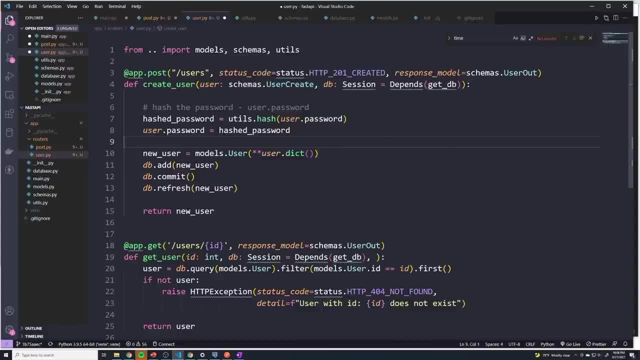 utils, And so, right there, we cleaned up some of our errors that we're getting, And let's see, we also have to import status from the FAST API library. So what we can do is we'll just go up here And I'm just going to copy this: 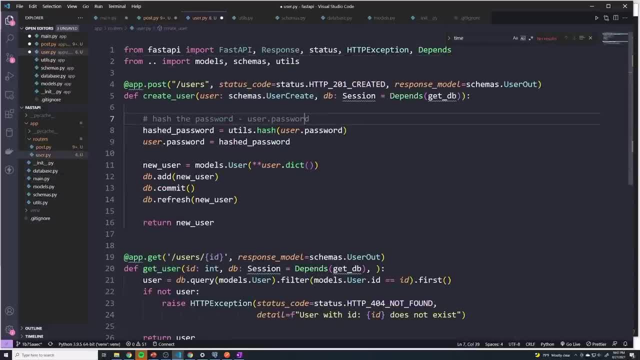 And right above this line, going to paste that in there. And the last thing that we need to import is from the database that we, from the database dot p y file we're gonna have to import, get DB and then from SQL alchemy. 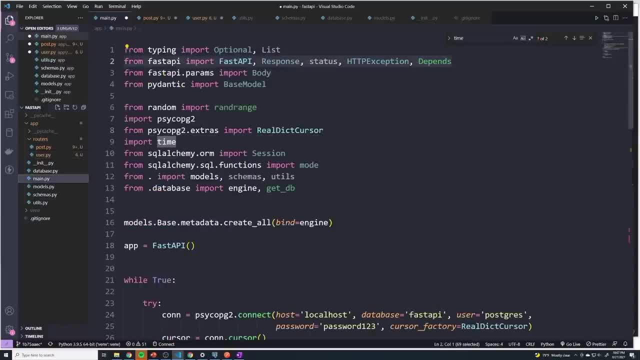 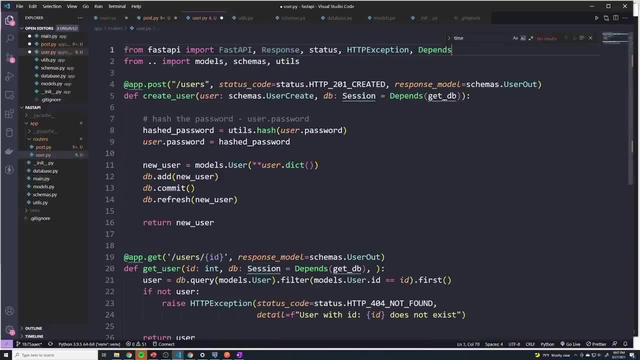 we have to import session. So if we go to our main dot p y file again the SQL alchemy code right here, we can just copy that And I'm going to import that as well. That's done. And then, finally, 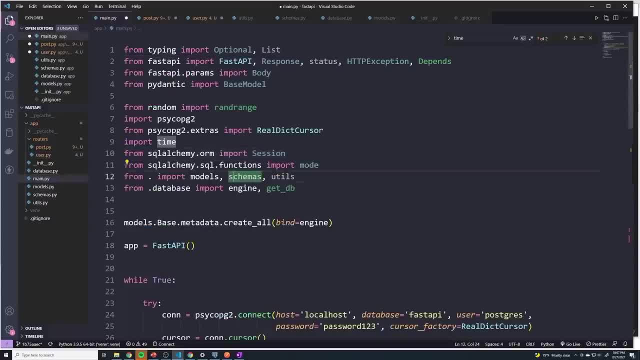 we have to get DB And if we take a look at our main dot p y file, the way we got that is, we're saying, from the current database file we want to import engine and get DB And keep in mind that the database file is not in the routers directory, it's in the app directory. So we have to go up a. 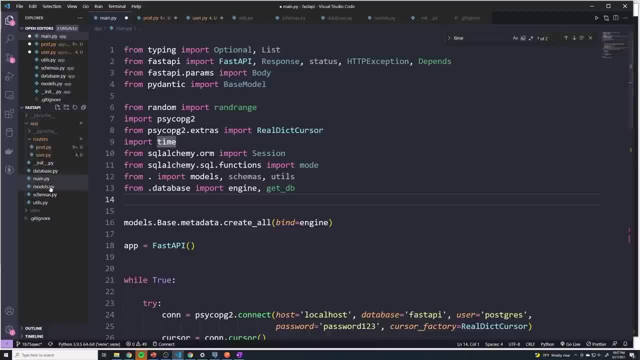 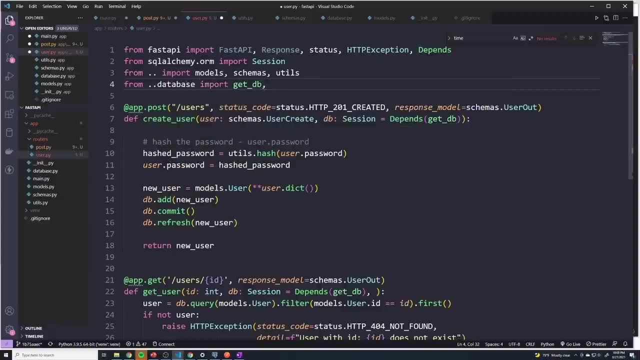 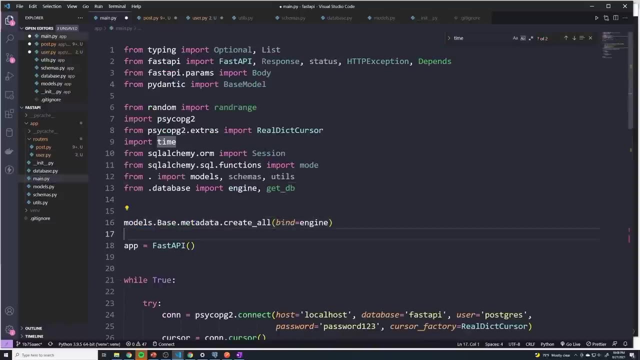 directory to access this file. So we just put two dots, pretty simple. So from dot dot database import, get DB, And we actually don't need to import engine. we're going to leave that here in our main dot p y file. Right, so now. 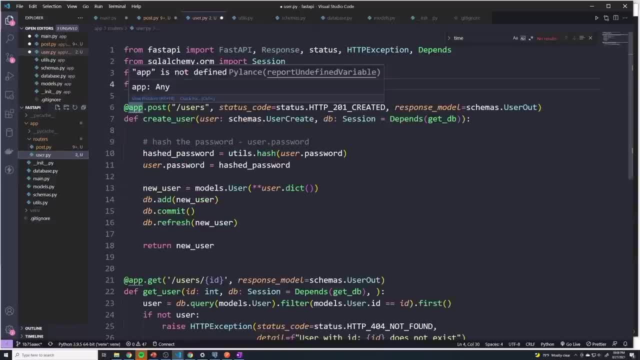 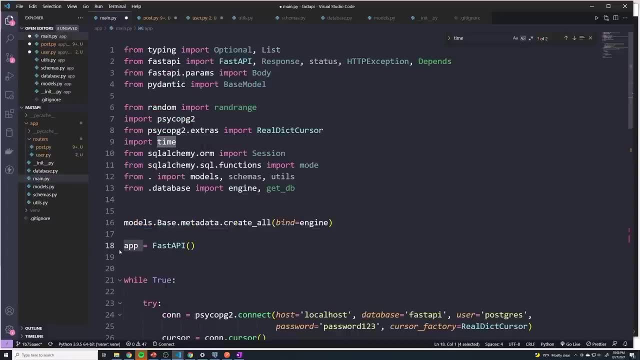 Speaker 1 that we got all of that. the last error that we see is that we don't have access to the app object, And so your instinct is to go to our main dot p y file and then import this, And that's not exactly. 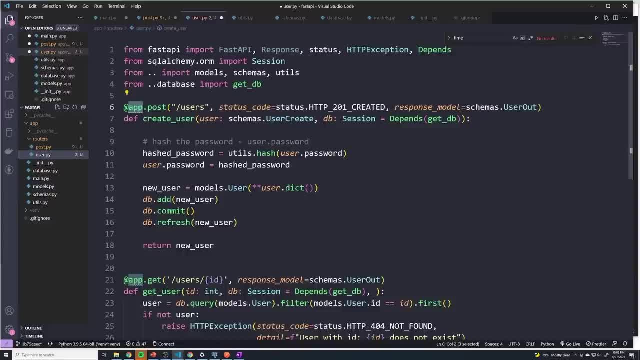 correct. Instead, what we're going to do is we're going to make use of the routers that I mentioned, And so from the fast API library, we're going to import something called API. first three letters, actually the first four letters- API router. 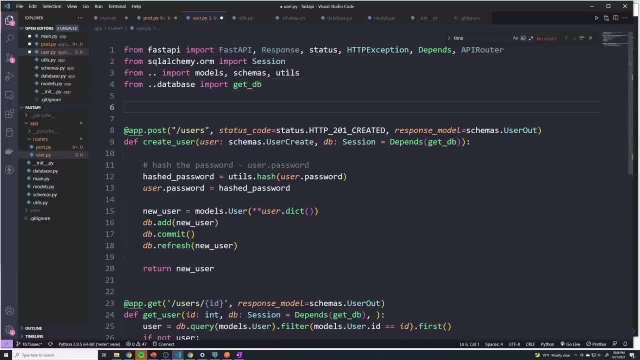 And then from here we're going to make use of the API router object. So we'll say: router equals API router. So we're basically creating a router object, And then what we can do is we can replace the keyword app, because we don't have access to that in this file, And 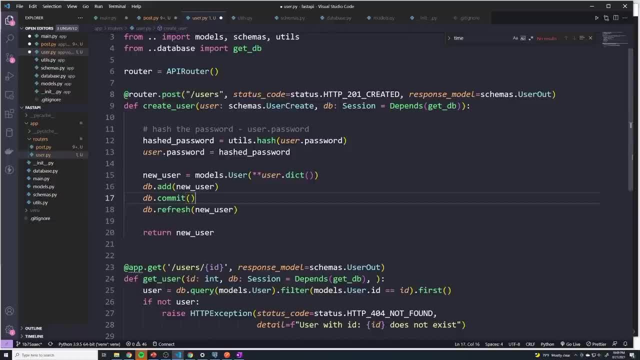 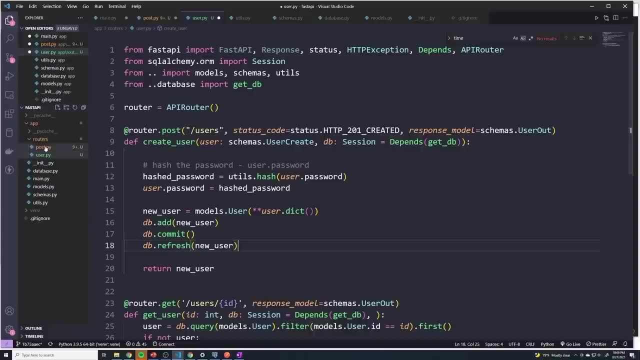 we just use the word router And you'll understand why we do this in a bit. So we've got those updated, And then we're going to do the same exact thing for our post op уров. So we have to get all of these imports. I'm actually going to copy most of these, because most of them are. 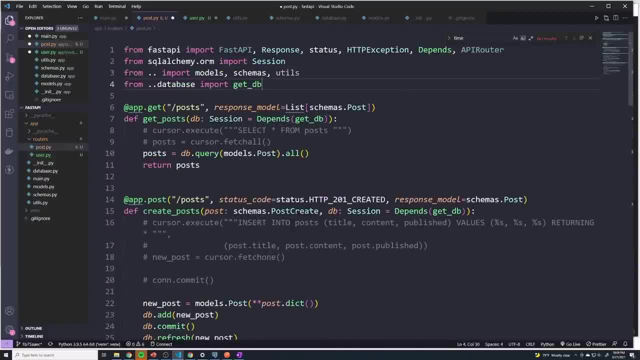 going to apply here as well. Speaker 1: have the only thing we don't need to. It's kind of complicated, but hey, hey, Hey, hey, Here in natural, here in natural, Put dot API. You do not need to add these fields here, Not only. 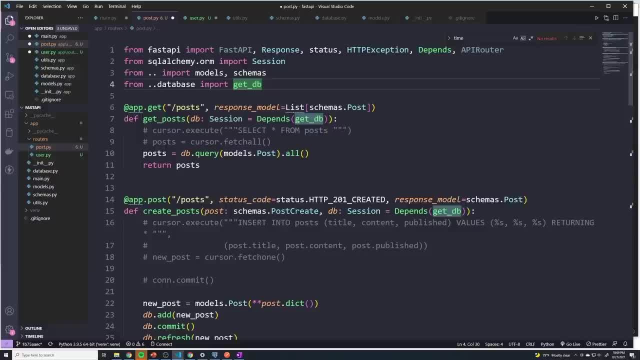 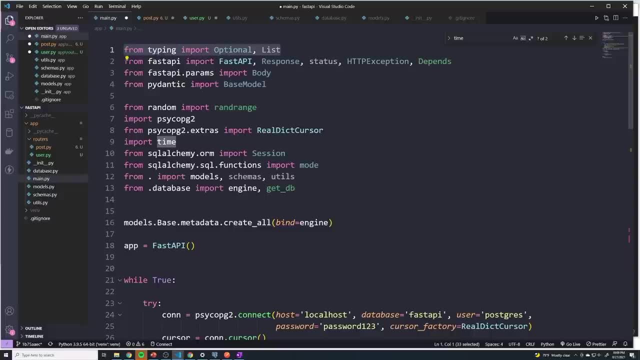 utils for sure. So we'll remove that And then you'll see that list is still getting errored out, And that's because if we go to our mainpy file, that's coming from this typing import. So I'm just going to copy that and paste that in there And it looks like we don't need. 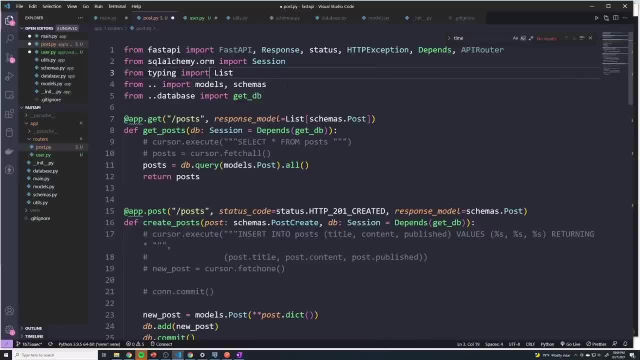 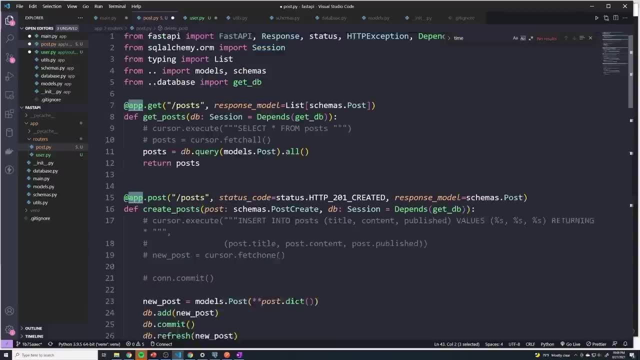 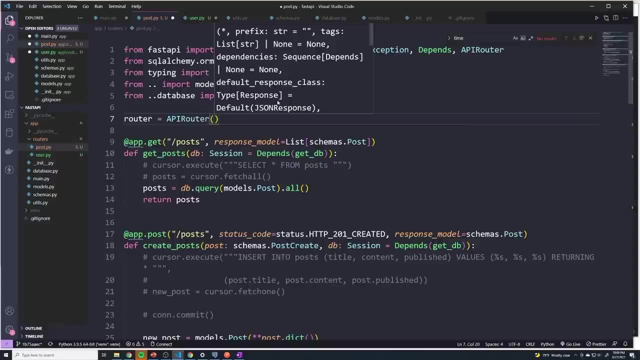 optional because it's kind of grayish. So that's just a VS code telling us that we're not using it in this file, And I think that should clear up all the errors, except for, once again, the app object. And so we'll do the same thing. We'll say: router equals API router, And then what we're? 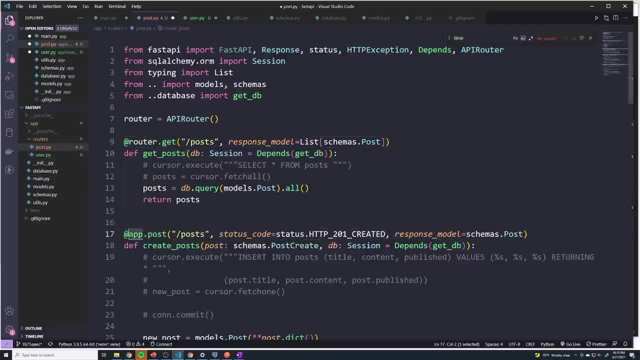 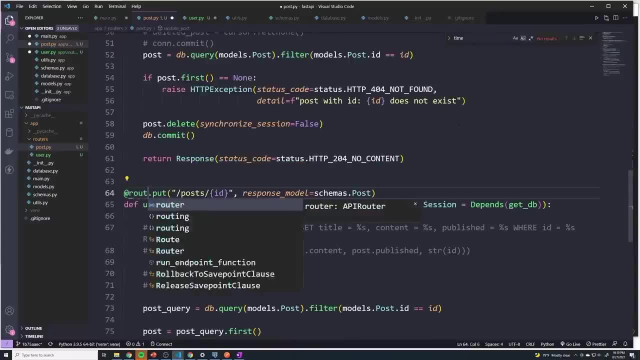 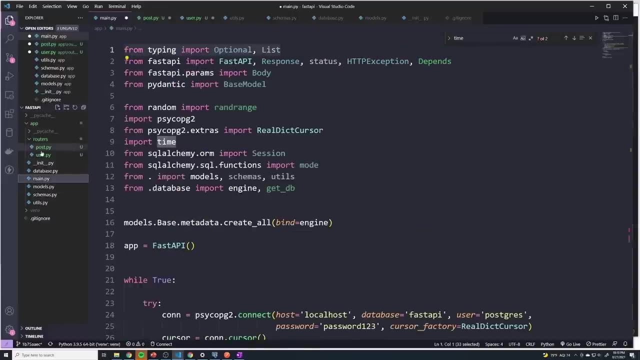 going to do is replace the word app with the word router, All right. and then, finally, we have to go to our mainpy file and actually make use of these routers, because you'll see that in our mainpy file, there's no reference to anything in here, So our API won't. 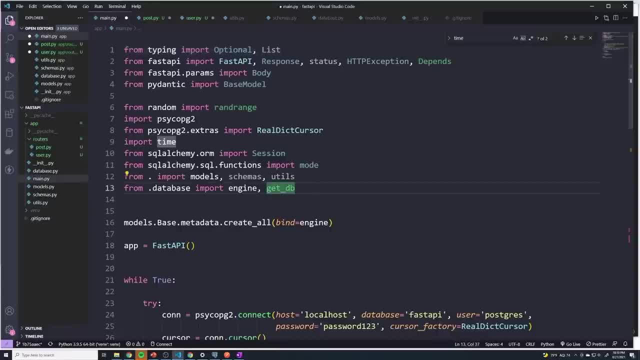 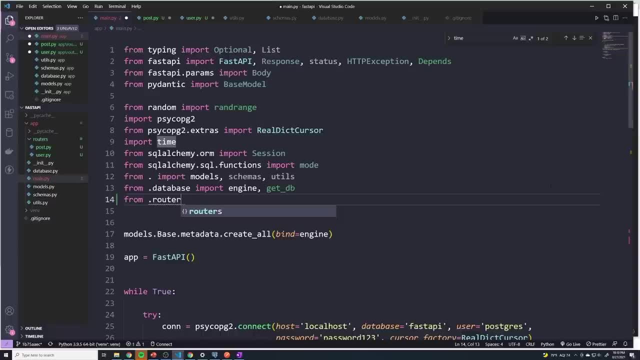 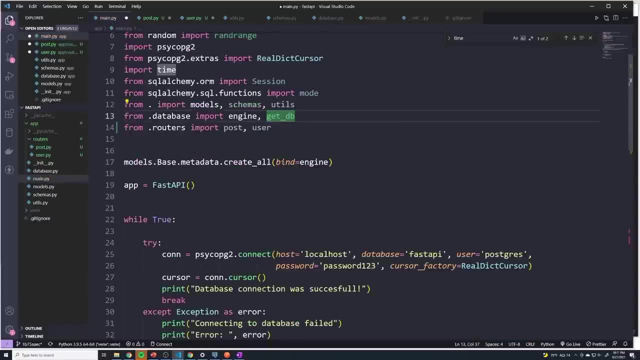 work if we try to run it now. So in our mainpy file, what I'm going to do is I'm going to say from dot routers, So from this folder we're going to import post and user And there should be plural routers, And I'm going to show you some magic that we're going to do. 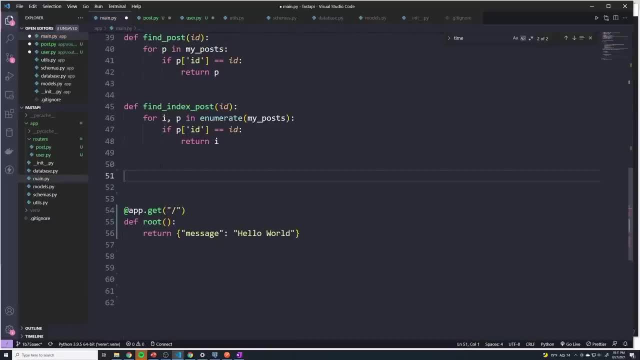 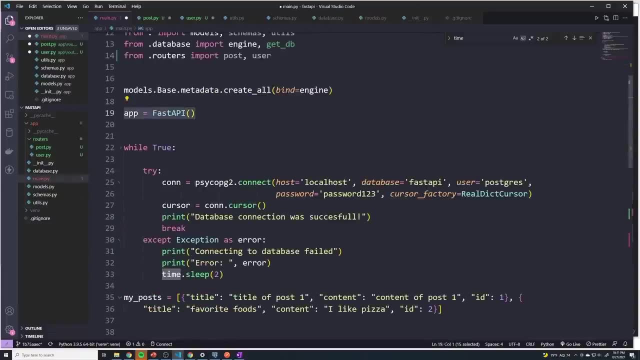 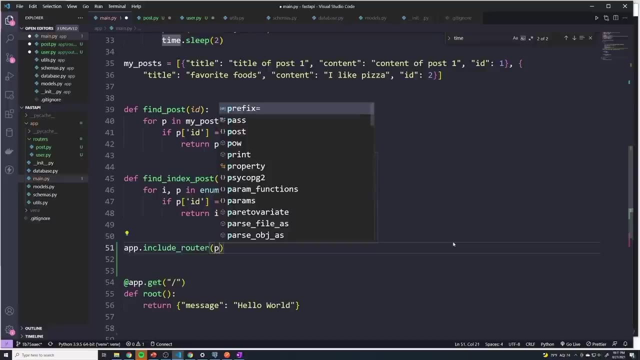 And so, above this route, we're going to say we're going to grab the app object right. this is once again our fast API object that we kind of do everything with. I'm going to say include router, And then we'll grab the post dot router, right. 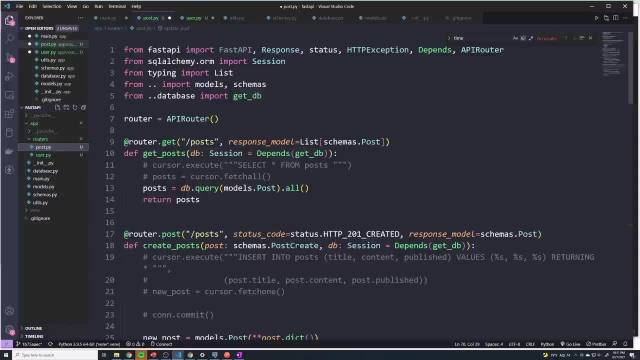 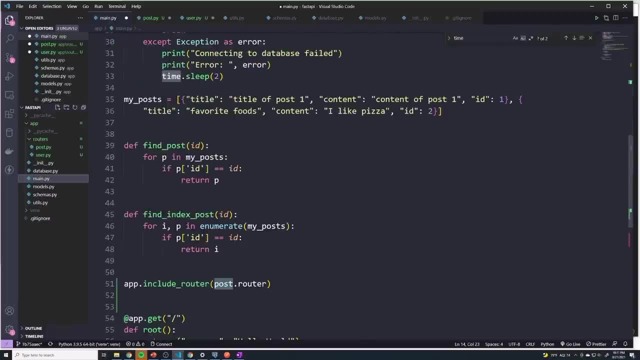 that's what we just imported. we imported post which is coming from here And we're importing this router object, And so what we've basically done here is, I have basically said, as we, you know, when we get a path, when we get a HTTP request, you know, before we had all of our path. 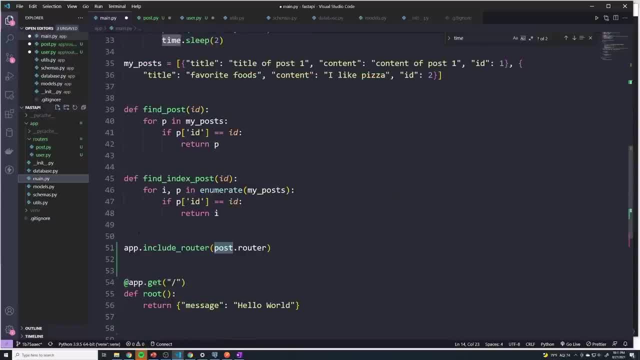 operations in here. instead, what's going to happen is, you know, we go down the list like we normally do, And so, as we go down our list, this is our first app object that we kind of reference, And in here it just says: I want you to include everything, I want you to include our post out. 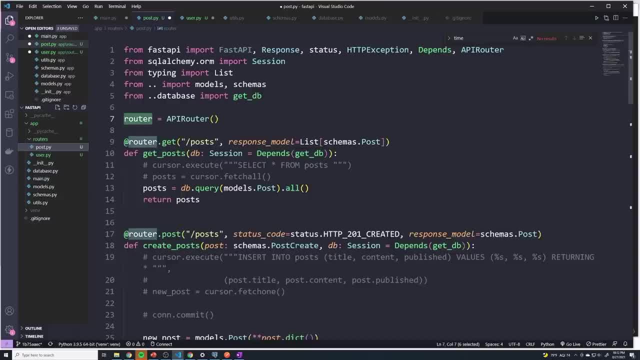 router And so the request will then go into here And it's going to take a look at all of these routes And it's going to see if it's a match Right, And if it finds a match, it's going to. 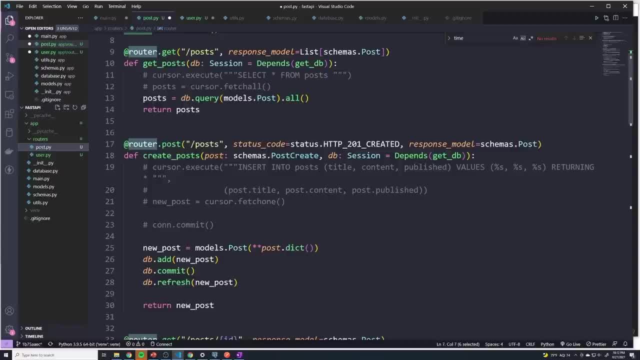 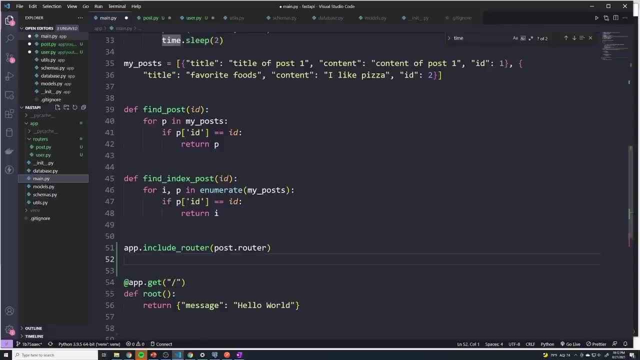 respond like it normally does. So that's kind of how we break out our code into separate files, we use these router objects And we can do the same thing with the user dot p? y. So we're going to go to main And then here. 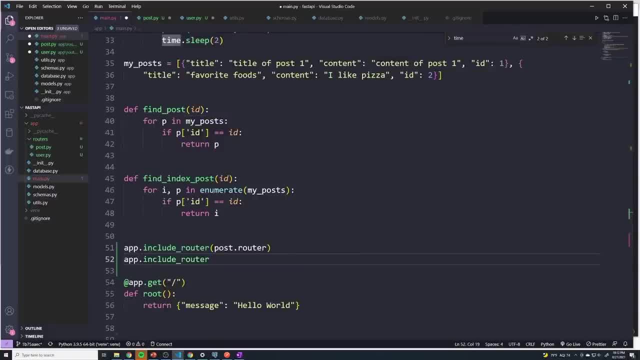 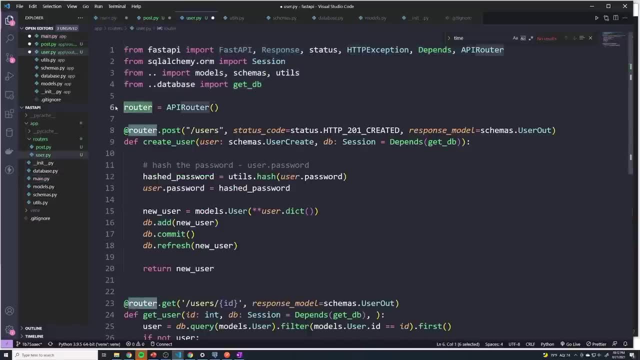 I'm going to type out the same thing. I'm gonna say: app dot, include router. And this time we use, we grab the user and then we do router again, And so, once again, all we're doing is we're just grabbing the router object from the user file And that's essentially going to import all of the 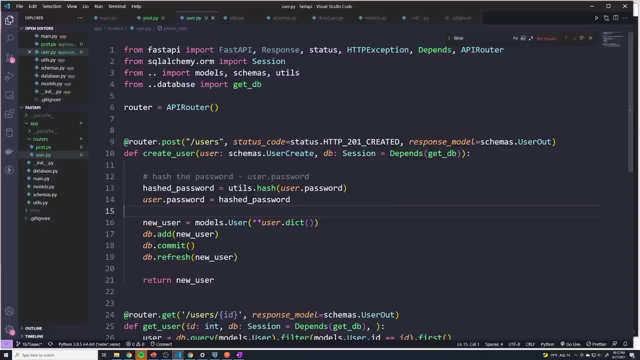 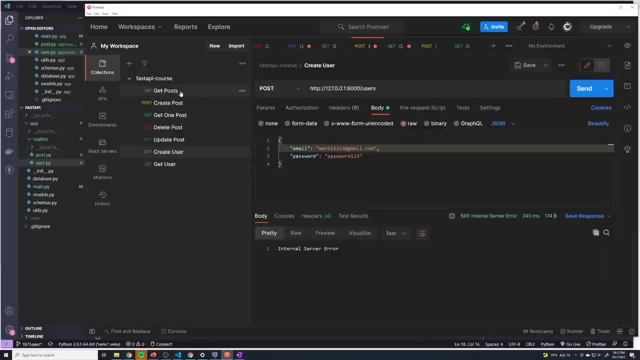 specific routes, And so if we save our code and then we just quickly take a look at the terminal just to make sure there's no errors, it looks like everything's working. Let's test this out now. So I'm going to get all the routes And then I'm going to go to the user And then I'm going to 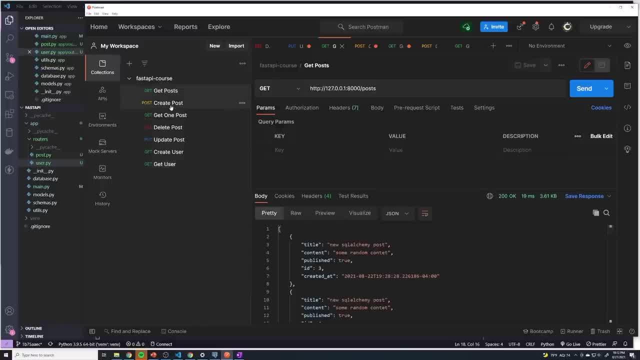 post. let's see if this works. It looks like it works. Great, Let's create a new post. Looks like it works. Get one post. Well, it looks like that post doesn't exist anymore, But if I try one, 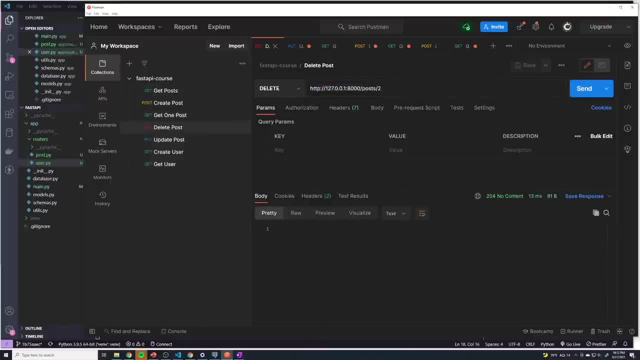 looks like it works, I will delete post with the ID of three. Great, we'll update post. create user: just put in a new unique email and then get user. So grab that user And we can see that every single route works. 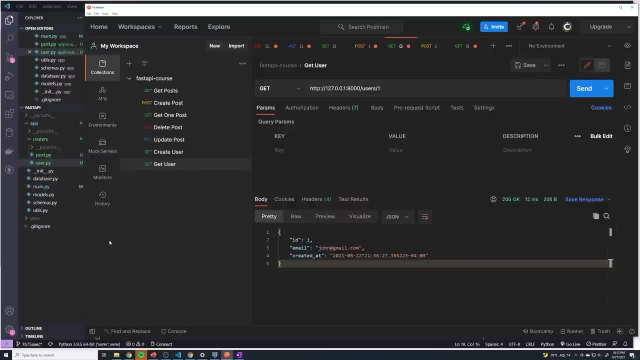 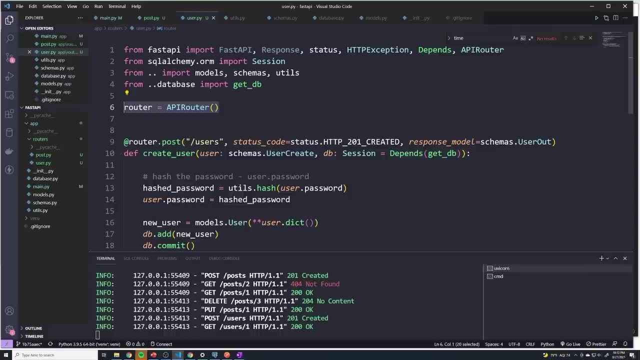 Perfectly So. we didn't change the functionality of our project at all in this video. Instead, all we did was we used a, a router object, to be able to split. split up all of our routes or path operations into different files, And then we import them just by calling app dot include router. 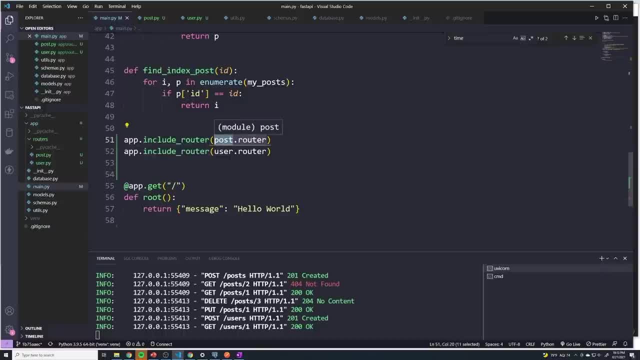 and then the specific router object of that file, And you'll see that our code looks so much cleaner now And, as our app and our API continues to grow, we can just add new files into the routers folder so that we don't continue to. 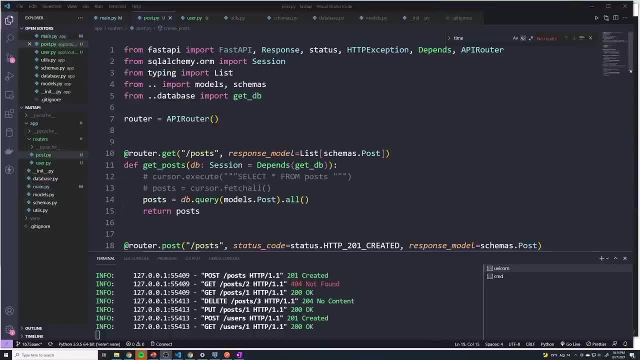 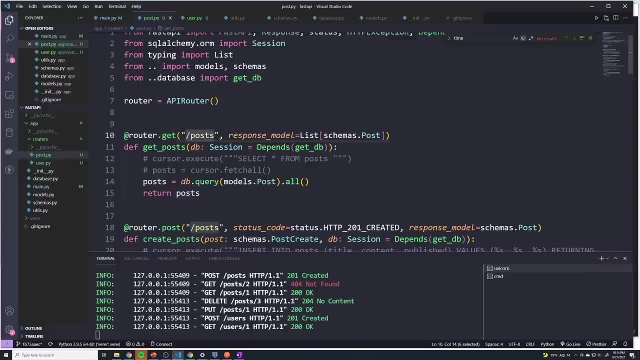 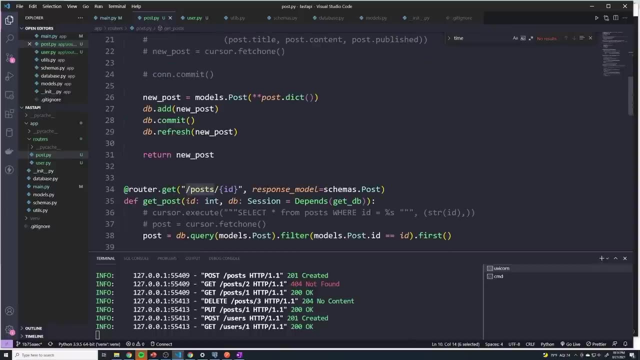 Clutter up our main dot py file In our two router files. you'll see that we use the same URL for almost all of our specific paths And so you'll see for the get route we'll use slash posts for the post. we use slash posts. From the get specific post we do slash post and then the. 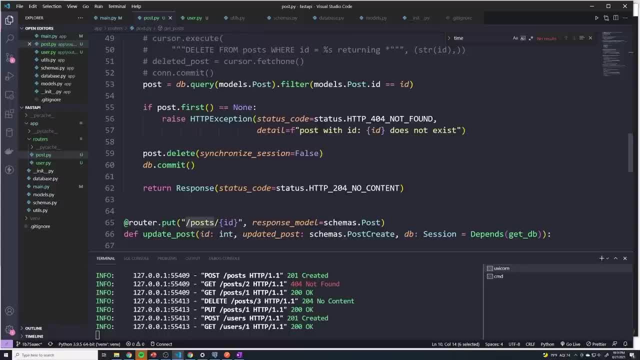 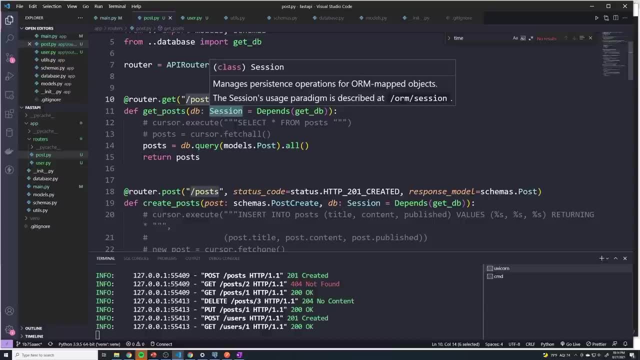 ID, and then the same thing goes for delete and and put as well, And I think it's kind of annoying having to continuously copy and paste the same exact path when it's pretty much just a copy From each one. So is there a way we can kind of remove this unnecessariness? It doesn't seem like. 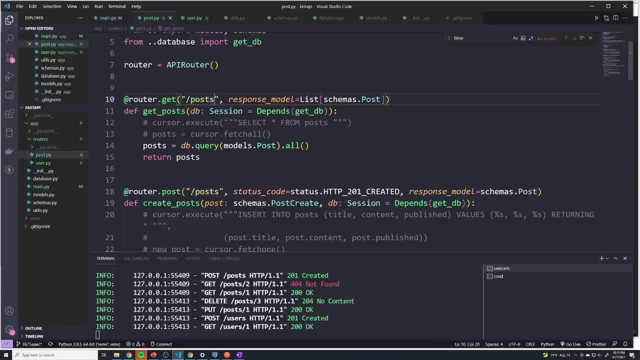 that big of an issue. But keep in mind that our API is very simple, right? Other API's could have very long, complex, you know routes that you know may not look as simple as ours, So they could have you know multiple things, right, So it could look something like: 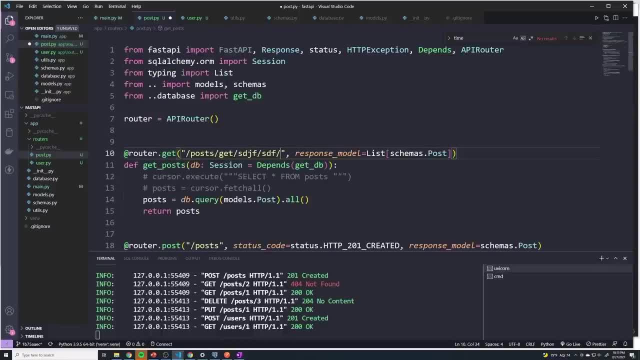 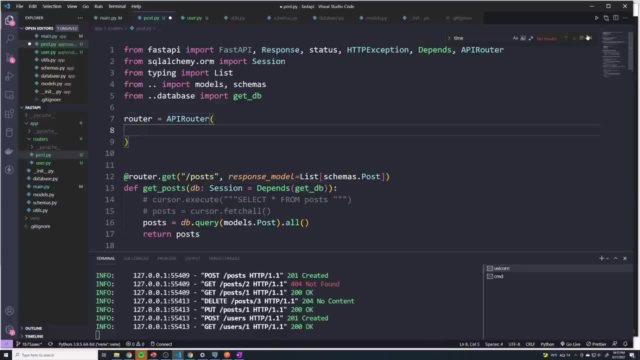 that, And then having to kind of copy and paste all of that every on every single route can seem a little unnecessary. And so, anytime you're working with routers, what we can actually do is we can pass in a parameter into the API router function or method, And so what we can say was: 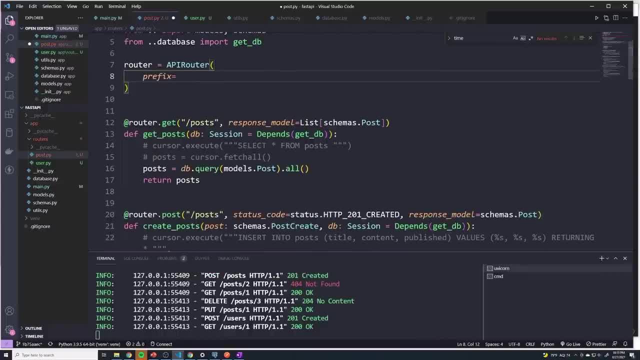 prefix And we're going to say that, since every single route in this file always starts with slash posts, we can say: prefix equals slash posts And so now, anytime you see a slash post, we can just remove that And just put in a slash. this just going to be a slash. 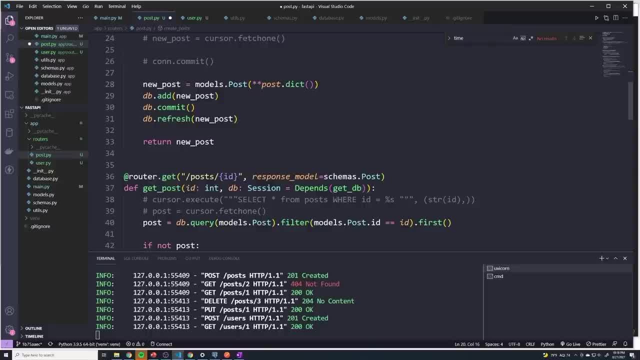 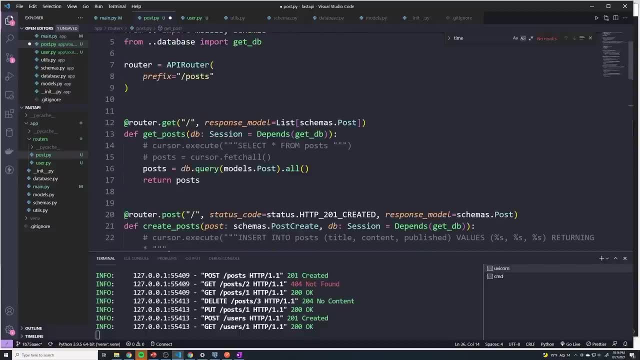 And then when it gets to slash post, slash ID. this is where it gets a little tricky, But once again, we just remove everything but a slash. And so what this is saying is that we're going to take slash posts And then we're going to append it with ID right, Because that's 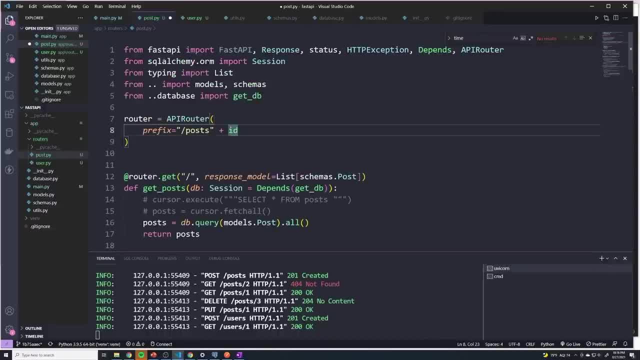 that's what this is saying. We're saying slash ID, So it's actually appending it with slash ID, So the final thing actually looks like it's going to look like slash posts ID, So nothing actually changes. It's just a simpler way to do that, And then we're going to take slash posts And then we're. 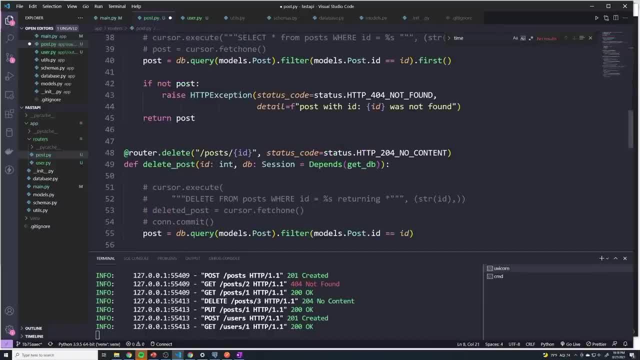 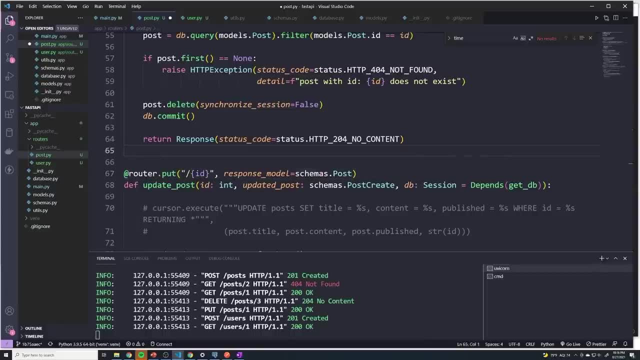 going to do things so that we don't have to write slash posts everywhere, And so we can. we can remove this and just do slash ID, And we can just do slash ID here as well. And we're going to do the same thing in the users file as well, because both of them start with slash users, And so we're going. 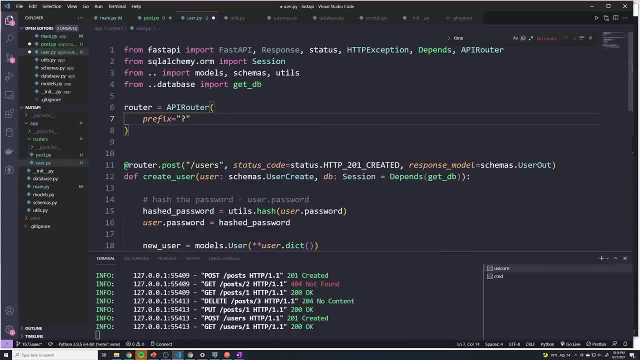 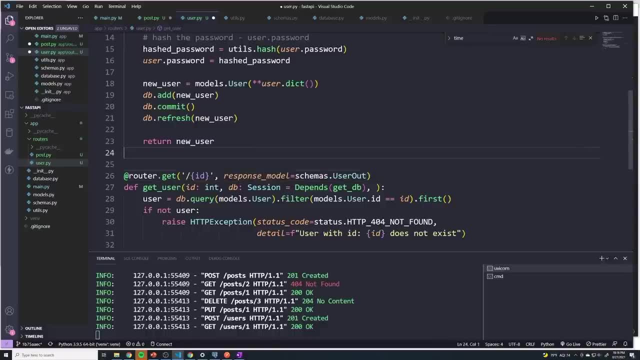 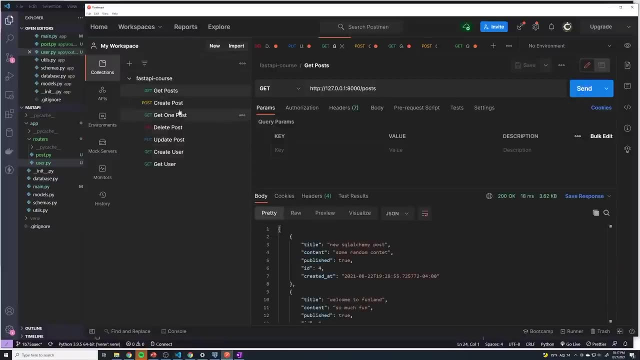 to put in a prefix here And we're going to say slash users, But this can just be removed to slash And this can be removed to just slash ID. Alright, and once again, we're going to test this out. We're just going to test a couple of routes. So if get routes, get posts work And if create 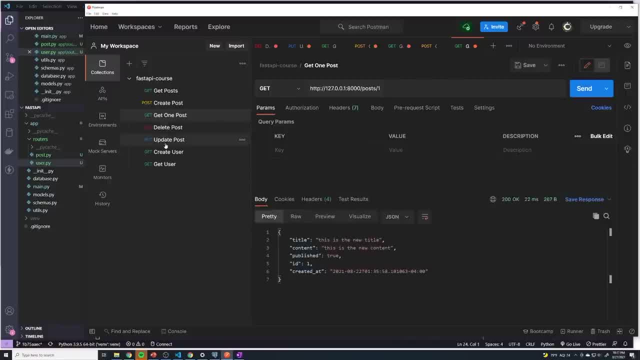 I will try to get one post that works perfectly, And then let's try creating a new user. we have to give it another unique email. Looks like it works, And then finally get user. we're gonna try this again And it looks like it all works. So you know, this is a completely optional step. 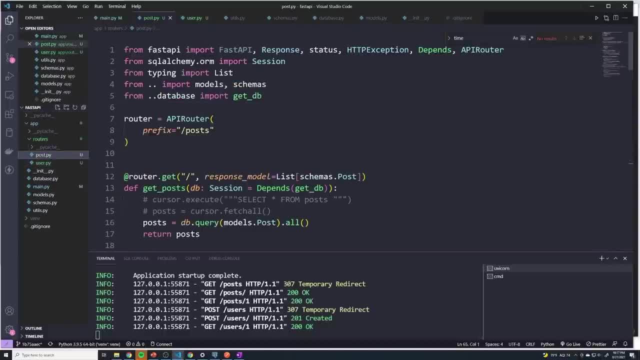 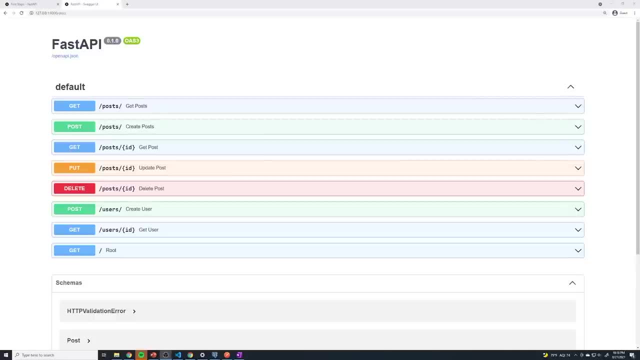 it doesn't change the functionality of things, But I think it does make it a little bit easier to read Because we've put the prefix up here so that we don't have to keep copying and pasting. Now, as I mentioned, one of my favorite features of fast API is the automatic documentation that 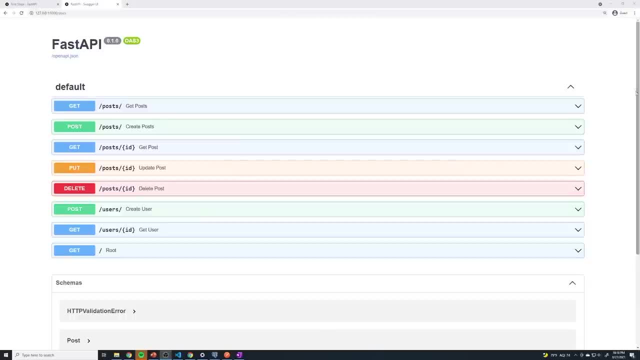 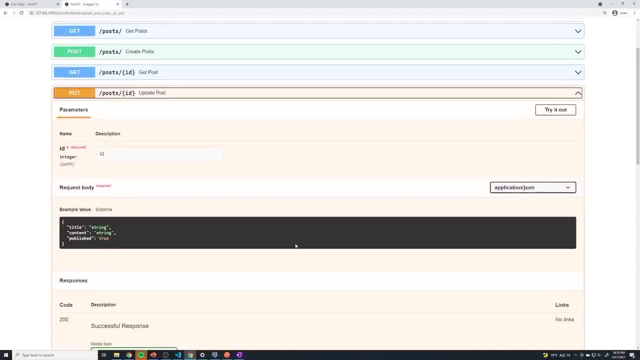 comes from swagger UI And so if you actually navigate to the URL but just go to slash docs, like I have, that's where you're going to see the documentation. Like I said, this is interactive documentation, So you can actually make requests from here. So 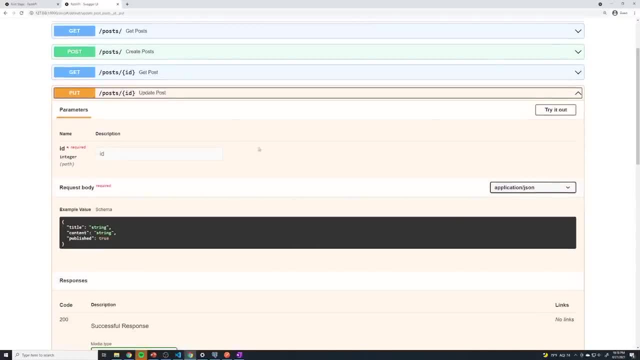 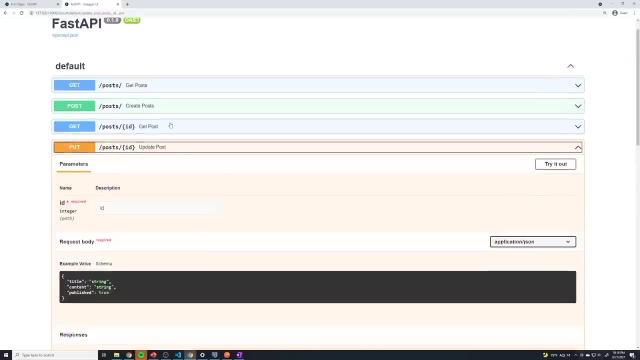 you didn't technically have to use postman for a lot of things. you can just test it out right here And it's going to do the same thing. However, I did also want to teach postman, But the reason I bring this up again is that you'll notice how we've got a couple of routes. 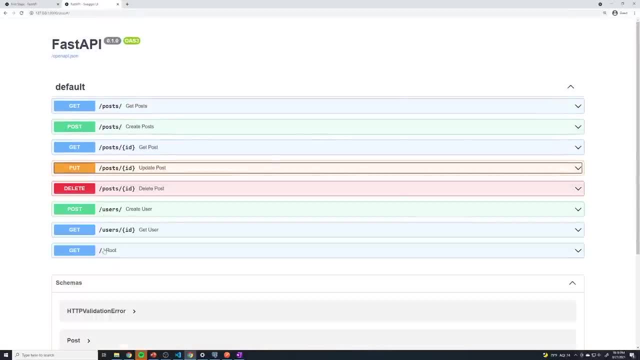 we're dealing with posts, and then we've got a couple of routes for dealing with users, And then we've got this random test one that we created when we were first learning about path operations, And what I would like to do is I would like to structure this documentation so that 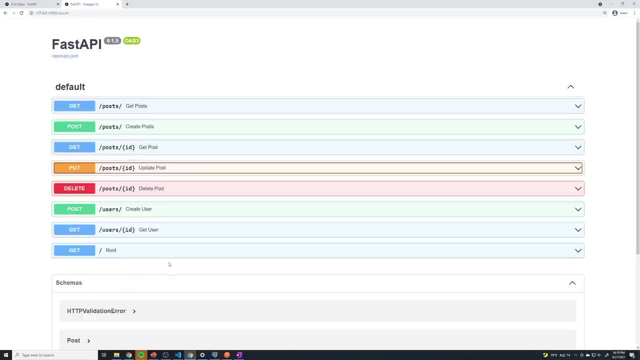 instead of kind of grouping them all together, we can kind of group them based off of the their responsibility. So I would like to create a group that handles all of the post operations, So all of these five right here, and then I would like a separate group that handles 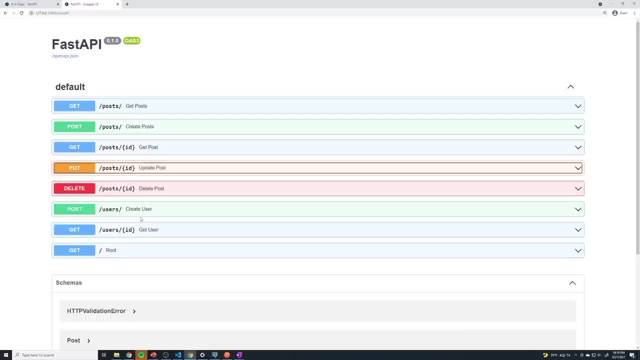 all of the user based operations so that it's a little bit easier for your clients and your users to understand what each one does by grouping them accordingly, based off of their specific action, And so I want to have a group that actually is titled posts and a group that's titled users. 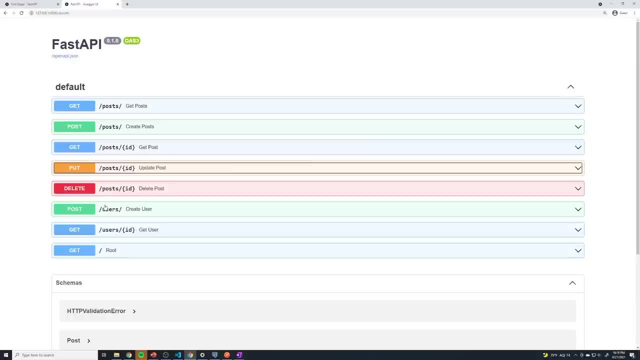 so that when they see that, they say: oh, the user section is going to be dealing with users and the post section is going to be dealing with posts And getting this fixed. our update in our code is super simple with fast API. So let's go to our fast API, go to our routers And if we go to 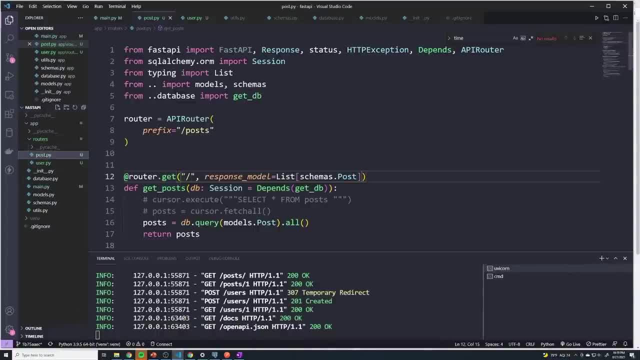 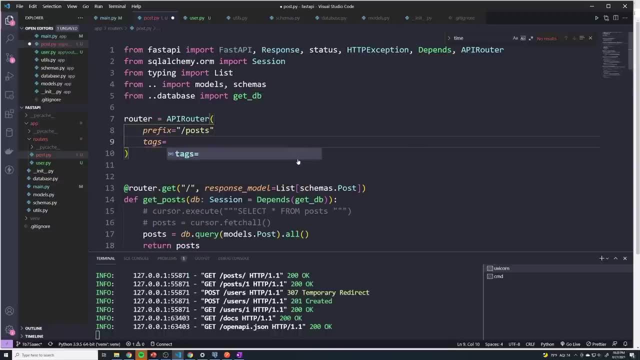 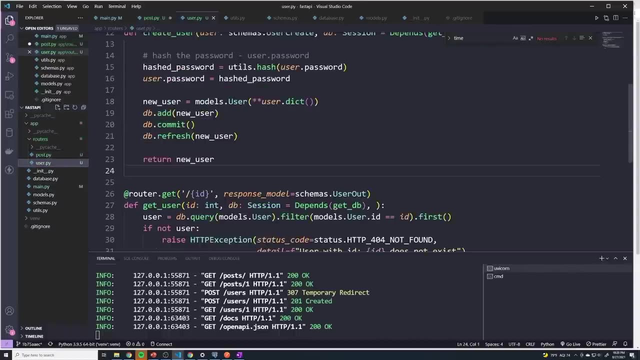 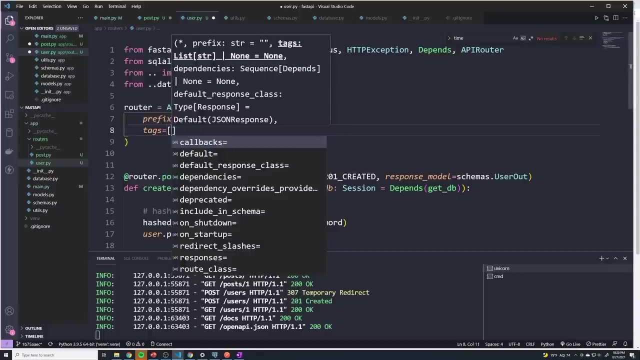 the post, that py, To add a specific group name. what we're going to do is we're going to go to name what we call. it's actually called a tag. So we say tags equals. We just say posts, And I forgot that comma right there. And we do the same thing for users. So we'll say tags equals users. 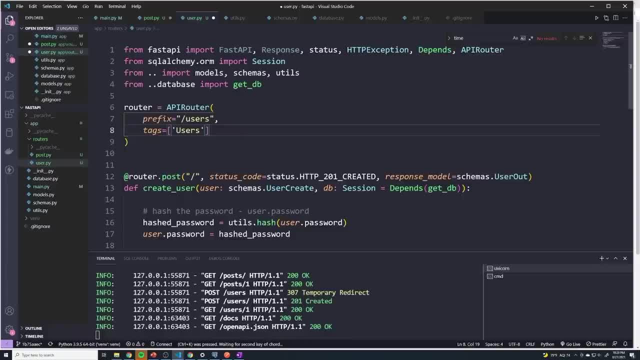 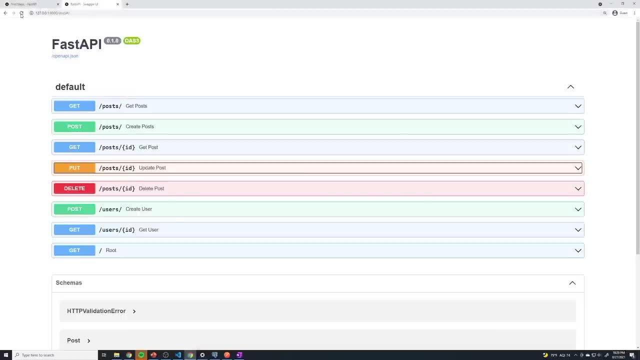 And you can see that this is a list, so you can pass more than one, But we'll save that And then I'm going to refresh this page. So now you can see that we now have these little titles, so that we can now group our specific. 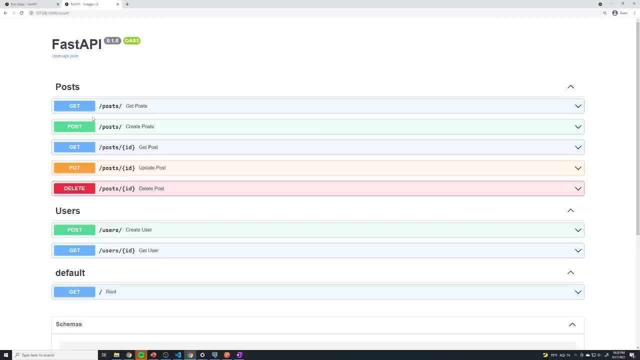 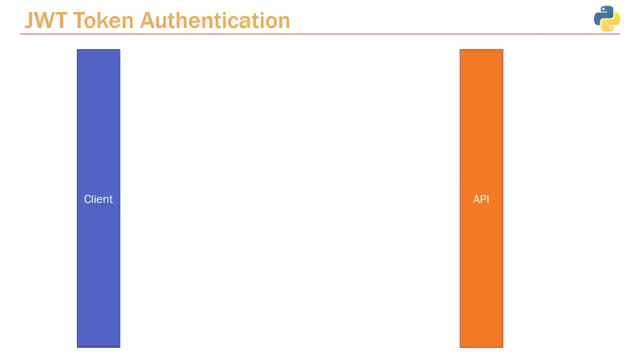 requests into categories, And so the readability of our documentation has improved tremendously. with essentially one line of code In this section, we're going to start tackling one of the most important topics when it comes to building out an API or really any application, And that is. 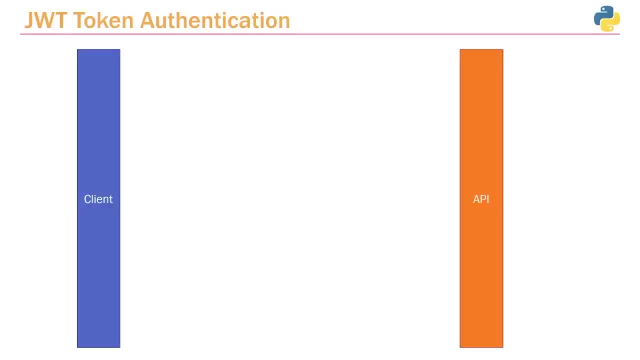 authentication. Now, when you're working with authentication on an API or any application, there's really two main ways to tackle authentication. There's the session based authentication, And the idea behind a session is that we store something on our back end server, or our API in this case, to track whether a user is logged in. So there's some piece of information. 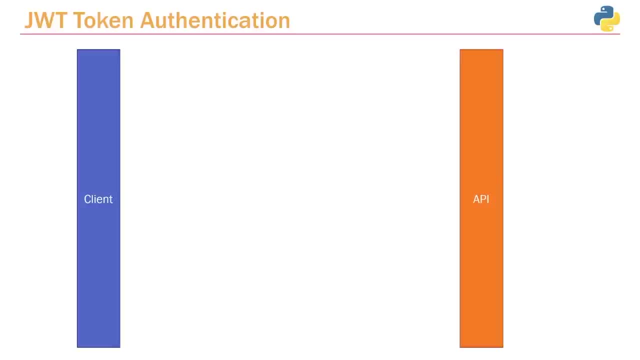 whether we store it in the database, whether we store it in memory, that's going to keep track of if the user has logged in and when the user logs out. So that's one way of doing things. The other way of doing things is doing is using JWT token based authentication. 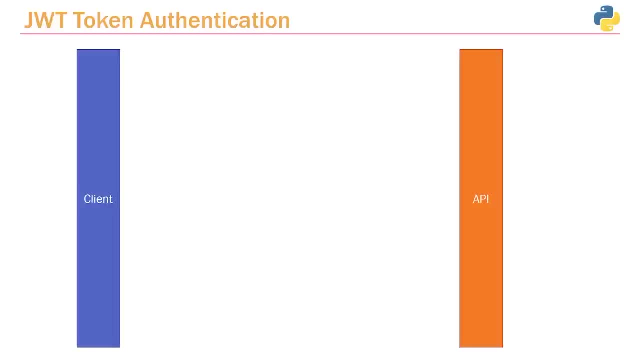 The idea behind JWT authentication is that it's stateless, And what I mean by that is that there's nothing on our back end, there's nothing on our API, there's nothing in our database that actually keeps track or store some sort of information about whether a user is logged in or logged out. 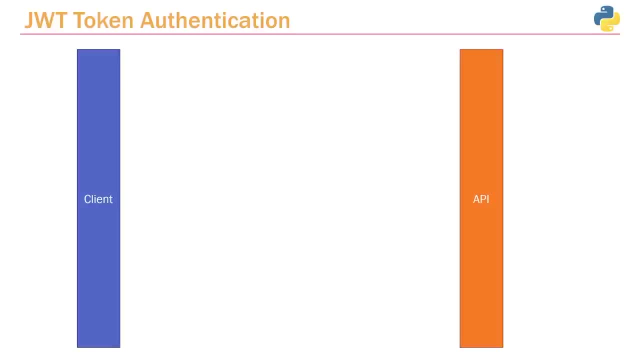 And you're probably thinking: well, how do we know that they're logged in? Well, that's the power of JWT tokens: is that the token itself, which we don't store in our database and we don't store in our API, It's actually stored on the front end on our clients- actually keeps track of you know? 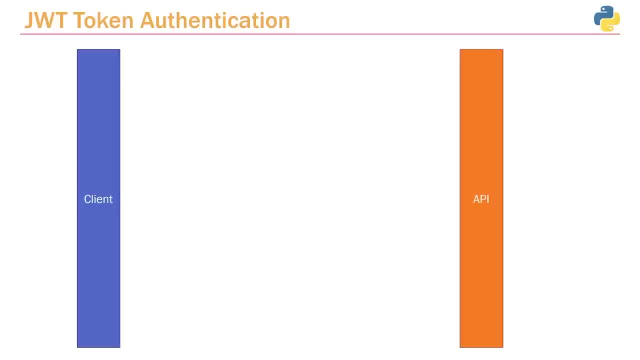 whether a user is logged in or not. And when I first started learning about JWTs, it was a little bit of a complex topic. it seemed like there were so many pieces that were in play. But then when you, when I, actually stopped to really understand it, I realized it's one of the simplest solutions. So 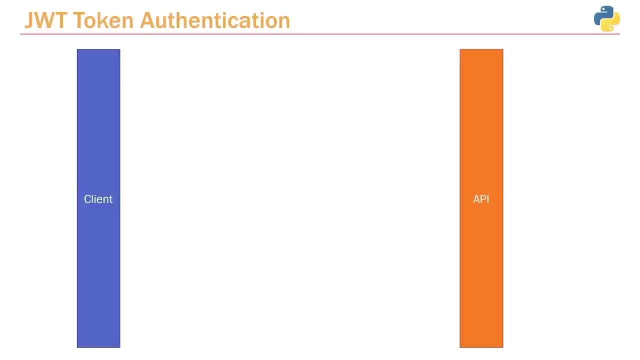 hopefully I can make this as easy as possible for you guys. I hope this doesn't end up kind of confusing you like it confused me at first. it really is simple And there's really only a couple of steps, But you got to really understand what a JWT token is and what we're doing on the front end. 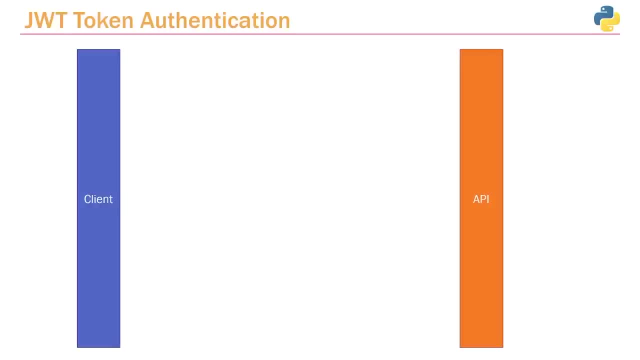 to make it so that we can actually use it as an authentication solution. So let's take a look at the flow for how a user logs in, how a user is essentially authenticated and then how a user accesses a specific path, operation, resource or endpoint by using the JWT token to ensure that. 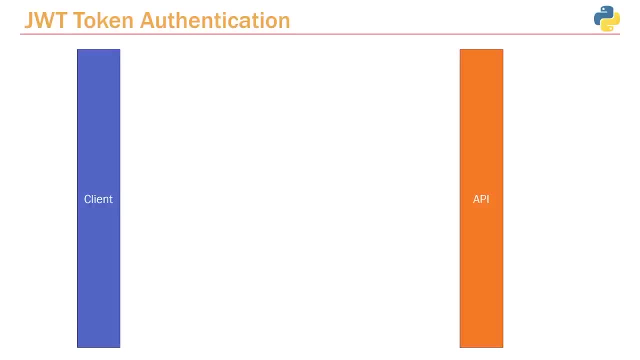 the API knows that we're logged in so that we can actually provide him that important information, And so what's going to happen is the client or the front end, whoever it is- they're going to try and log in. So what we're going to do is we're ultimately 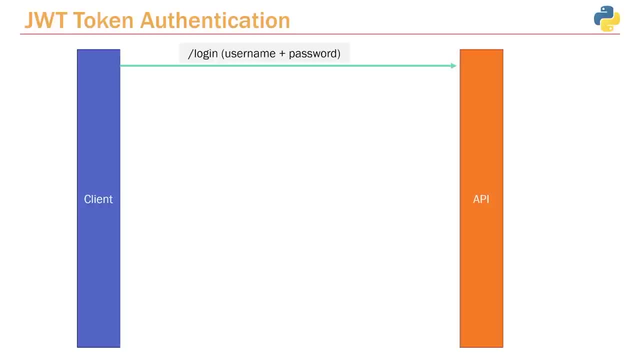 going to create a path operation called slash login And the the client is going to pass the username and they're going to pass in the password. So whatever their credentials are, so it doesn't technically have to be username and password, It can be email and password. 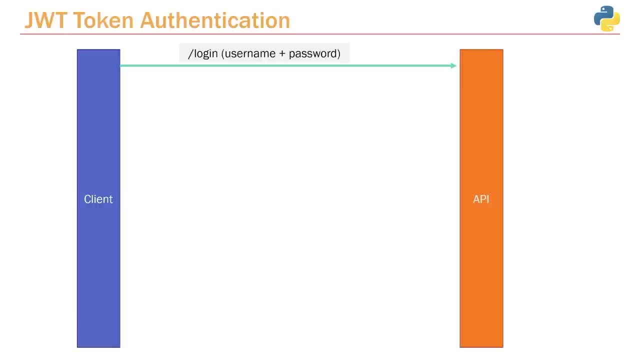 it can be whatever information that you want. So, technically, in our application, it's going to be email and password, because we don't have usernames- I guess we mostly just have emails- but they provide their credentials, And so, after we get their credentials, what we're going to do is, first of all, we're going to create 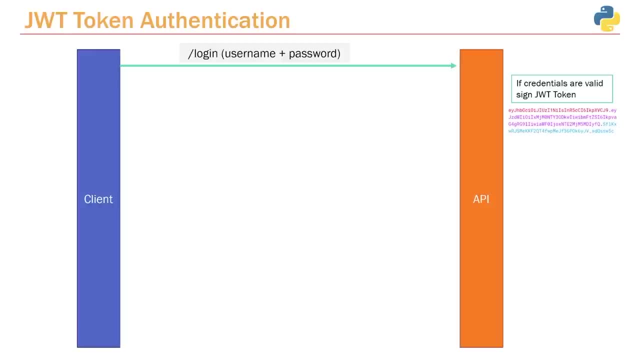 well, first of all, we're going to verify if credentials are valid right. So if the credentials are correct, if the password matches the, if the username and password match with the account, we're going to create this JWT token. And we haven't talked about what the JWT token. 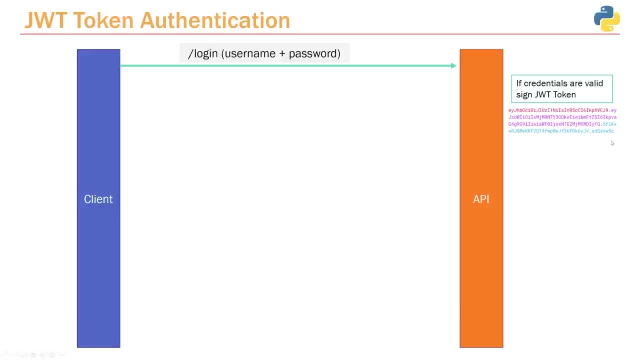 is, So don't worry too much about it, But I've created an example token right here, And so you're probably thinking it just looks like a bunch of gibberish And for the most part it is So moving forward. I want you to think of this as nothing more than just a string. 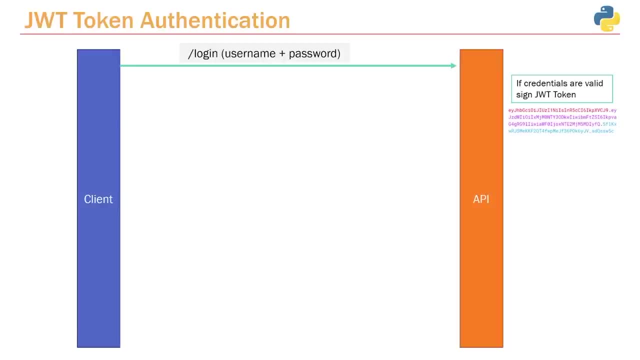 you know, just a regular string in Python. That's kind of fundamentally what it is, But there's a little bit more information embedded in it. But think of it as a string from the perspective of the client. the client doesn't know what the token is and it never. 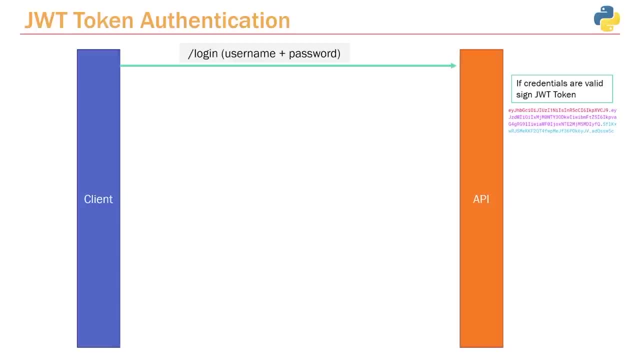 cares- really the only the API cares- what's actually in the token and what it means, And so we'll send a response back with the token. And so now the client has the token, And so he can start accessing resources that require authentication, So anytime he wants to. 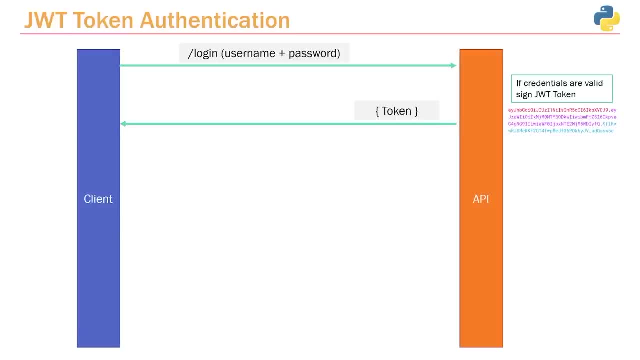 you know, let's say our application requires a user to be logged into retrieve posts. what he can do is he'll send a request to the slash posts endpoint, But he also provides the token in the header of the request. And you may not know what the header of a request is, But I'll show you, guys. it's very simple. 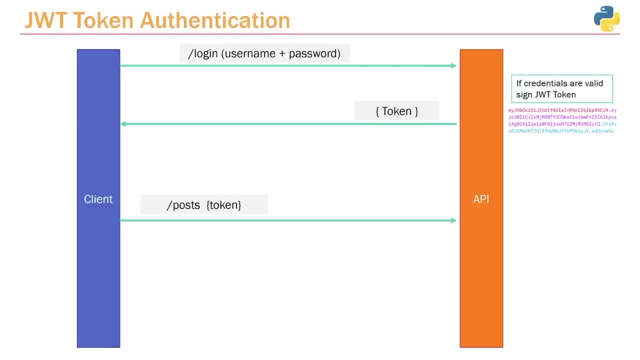 You can just think of it: it's somewhere in the payload of the request And so he sends that. And what the API is going to do, our fast API is: first of all, it's going to verify the token is valid, And there's a couple of different steps needed to actually verify if a token is valid, And we're 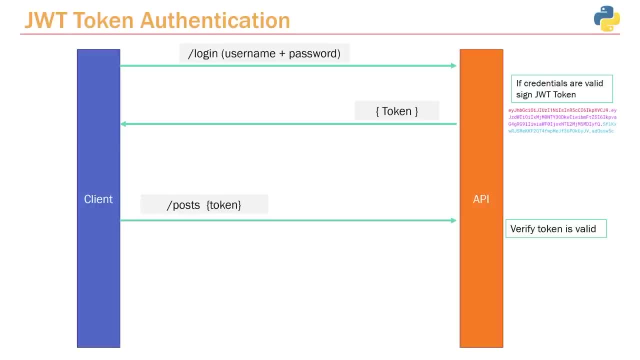 going to cover that in the next slide, But just know that the API just checks: hey, is this a token? And if it is, well, then he just sends back the data And that's it. Our authentication system is dead simple. You provide your credentials, you get a token And then anytime. 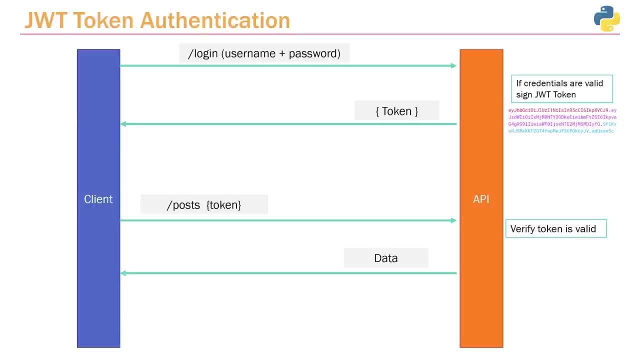 you want to access anything that requires you to be logged in, you just send the token in the header And that's it. So hopefully this wasn't confusing. Hopefully you guys see the simplicity in the solution. The API doesn't actually track anything. There's no information. 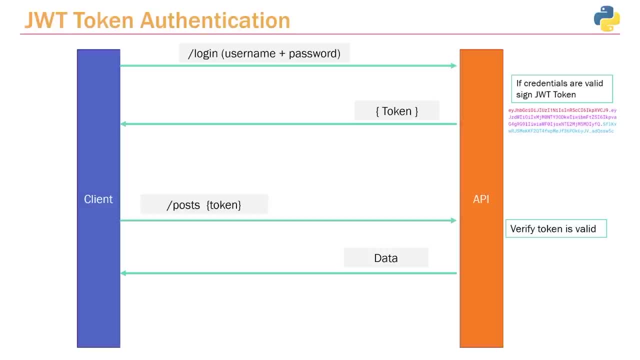 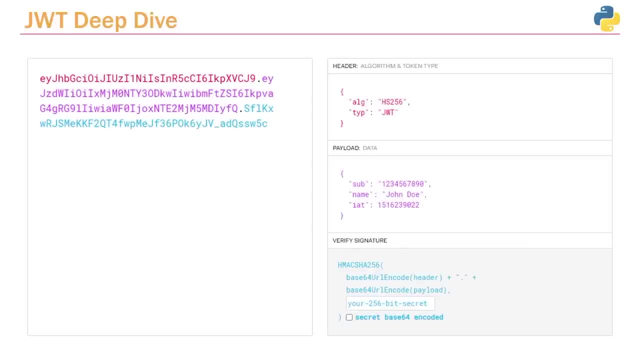 being stored on the API. Instead, the client just holds on to the token And he provides the token. So if we verify that the token is valid, that's all we have to do. So let's break down what exactly a JWT token is And what are the components that make up a token. And so I've got an example: token. 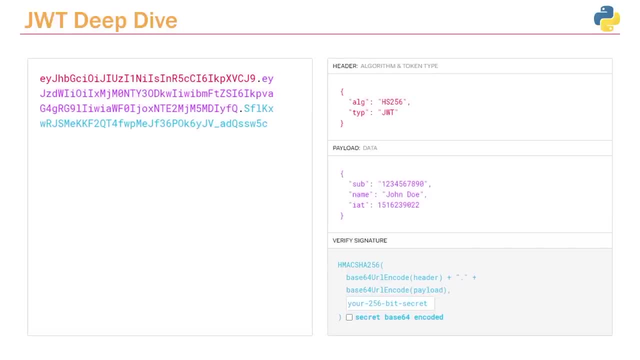 right here, And this is kind of the same piece of text that we saw in the previous slide, And so it once again just looks like a bunch of cryptic characters just jammed together, And that's kind of what it is. It looks like it's encrypted, But keep in mind, it is not encrypted. This is. 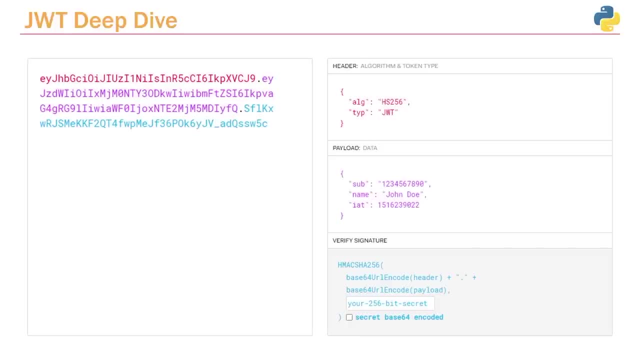 important to understand, And we're gonna make sure I drive home this point. it is not encrypted, But this token itself is made up of three individual pieces. The first thing is the header. So the header includes metadata about the token, And so we're actually going to sign this token, So we're 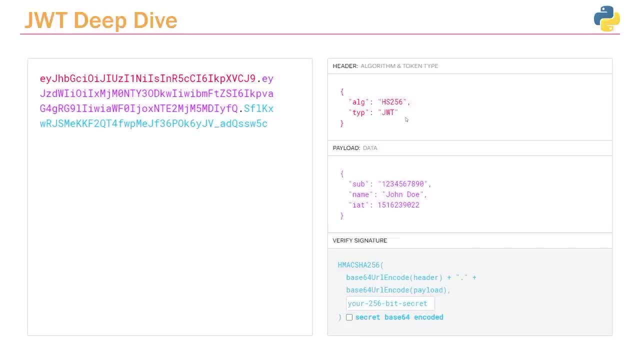 going to think of it almost like hashing the token, And so we have to specify the algorithm that we're going to use. So in this case the default is HS 256.. So we've included that in the metadata And then you can see the type is set to JWT. So this is a JWT token. So that's why the 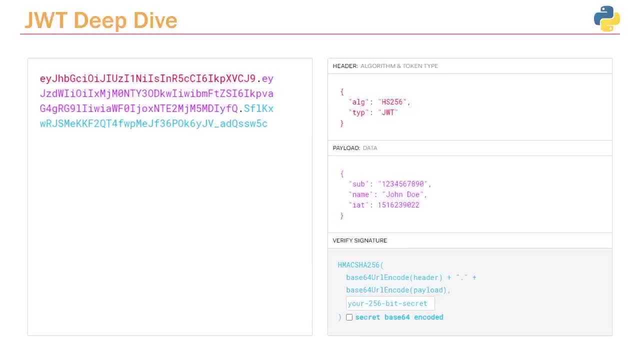 type is set, So the metadata is going to be the same for all of our tokens. This is just kind of fixed. don't worry too much about it. it's not really that important. we don't really ever touch it. Now the payload is a little bit more interesting. So the payload of 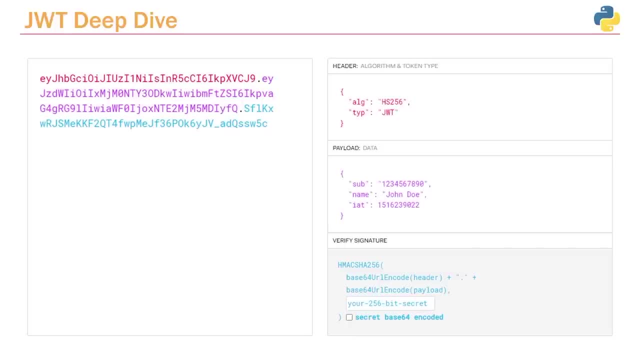 a token is ultimately up to you. you can send absolutely no payload. you can send any piece of information that you want to send Within the payload. you can include anything that you want. However, you want to be careful with what you put in the payload, because it's important to 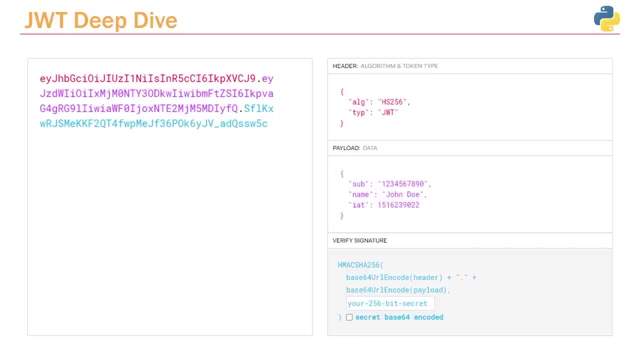 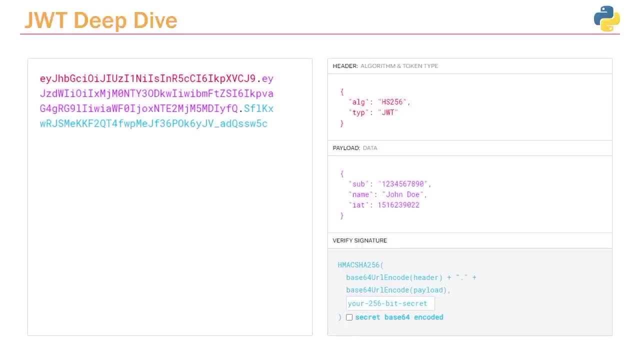 information you want. you don't want to put any passwords or secrets or anything like that. Instead, you want to stick to some very basic things. So very common things that we put in the payload are: what is the ID of the user right? So when I log in, I normally our API. 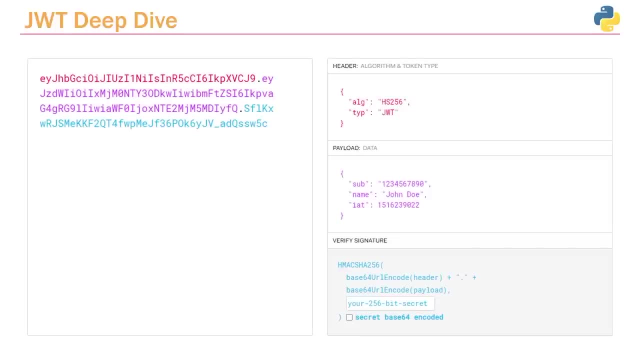 is going to create a token and then embed my user ID into the token so that, when I asked to get all of my posts the, the API will be able to take a look at the token, verify it's correct extract to the payload and it'll automatically know the ID of the user that requested this. 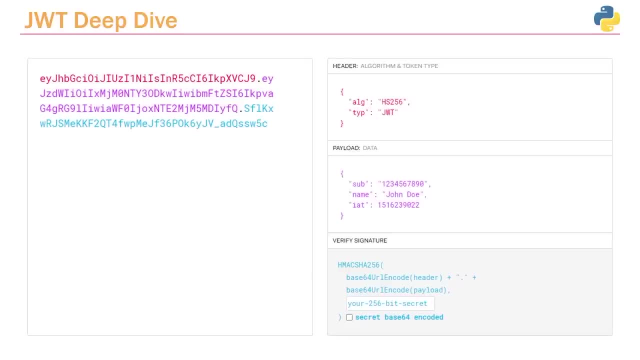 But we can include other things. we can include the user's role. So are they an admin Or are they just a? are they a privileged user? Are they a regular user? we can technically include any information. One thing to keep in mind is that anytime we need to access anything authenticated, 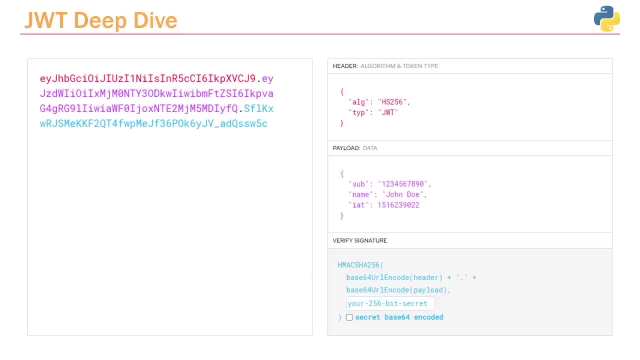 we have to include this token. So if we jam a lot of information in there, well it's going to increase the size of our packet And that's going to be a waste of some bandwidth. So you don't want to jam too much information. just a couple of small things here. 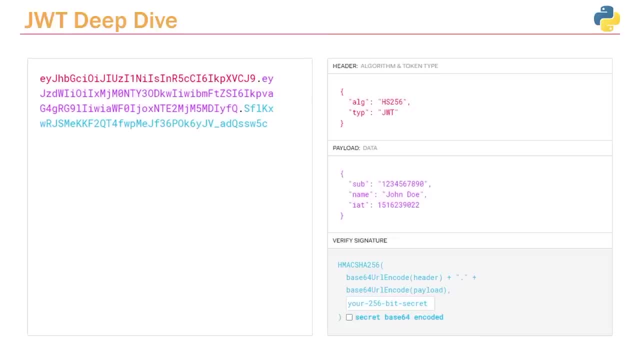 or there, And then finally we have a signature. So a signature is a combination of three things. We've got the header, so we take the header that's already in the token, we take the payload- that's already in the token, And then we add our secret, So there's a special 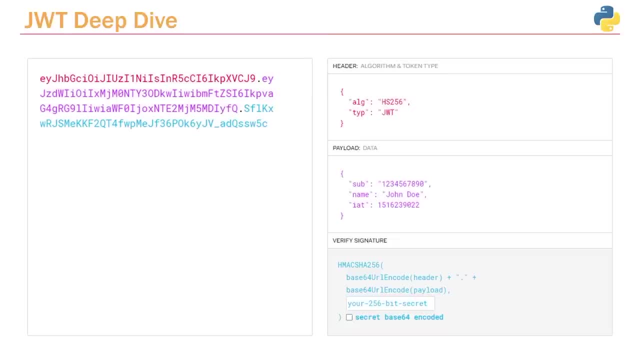 password that we're going to keep on our API. This is only on our API. our clients will not know it, no one else will know it, And it's probably the most important thing to our whole authentication system. So you don't ever want the secret to get out. But we take those three things. 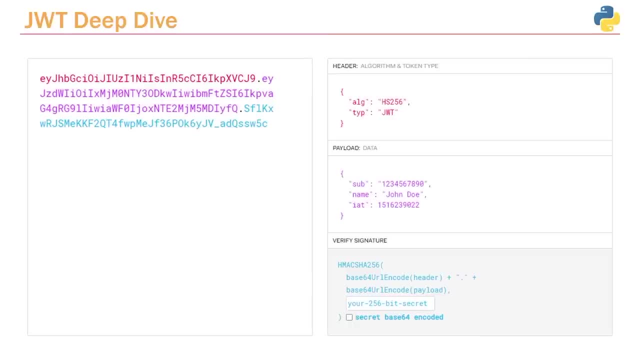 the secret, the header, the payload, And then we essentially take that information, pass it into the signing algorithm, which is the HS 256.. And then it's going to return a signature, And this signature is important because we're going. 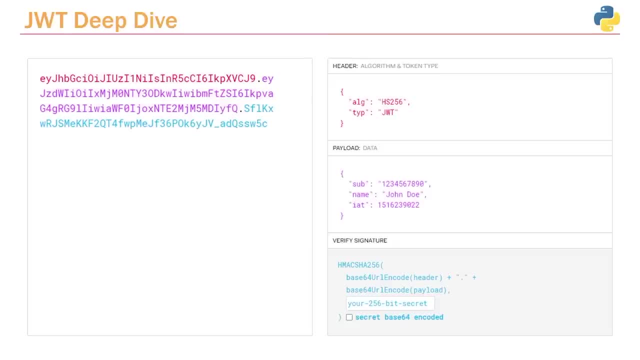 to use this to determine if the token is valid, because we don't want anyone else tampering with our tokens. we don't want them changing data. You know, I don't want some user to log in and then just start changing numbers in here to make it seem like it's a different user. 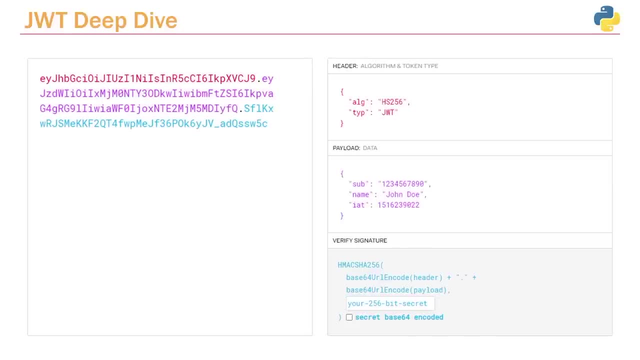 because then they can potentially access other users information, And so that's why we have this signature. It's just to make sure that we have the signatory And then we have a signature, and then to make sure that no one has tampered with our specific token. And so you know, I just 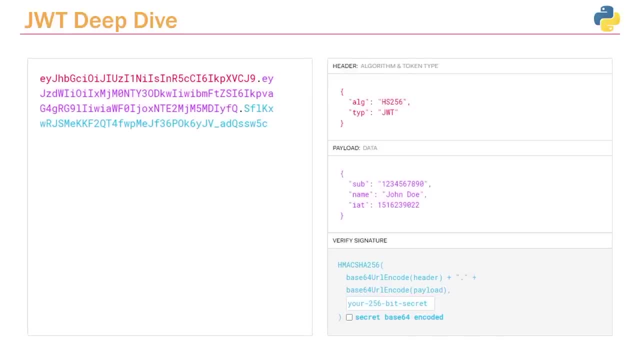 want to drive home that same point. First of all, there's no encryption, So anyone can see the data. the signature is just there for data integrity, And what that means is no one has changed it. That means all the data that we have in there is still what it. 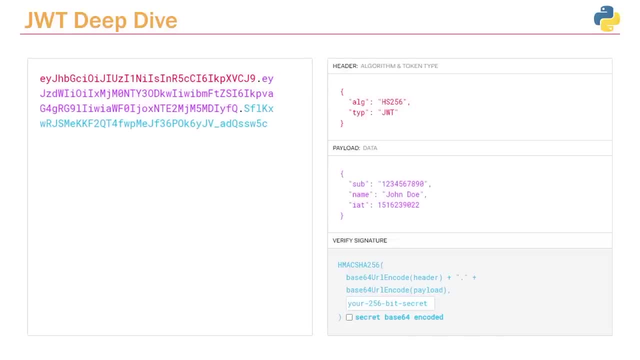 should be. No one has messed with the data Right And if you're still confused as to what a signature is, we're going to take a look at how signature work, why we use them and how they ultimately help us detect if someone changes any of the information. our 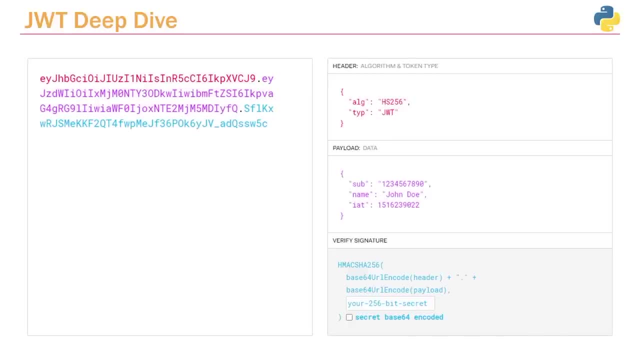 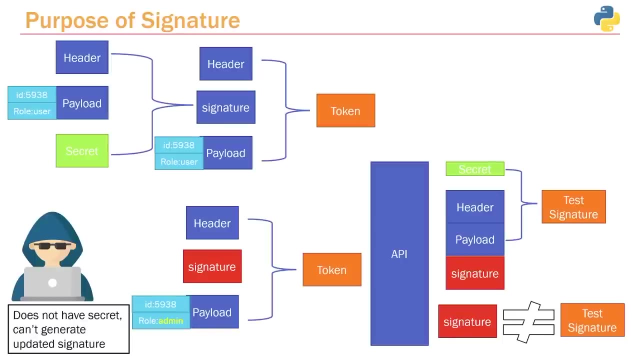 token in the next slide, And then I think at that point you guys will see it's not really a complex concept And once you get that, you'll see that the whole authentication process is fairly simple. Okay, guys, so we're going to do a deep dive into why we need the 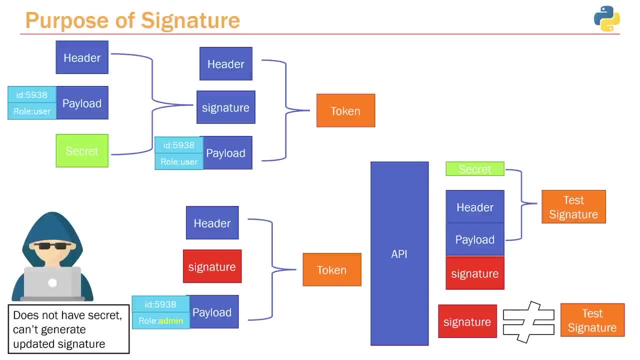 signature within the token And you'll see this. this slide may look a little complex. there seems to be a lot of boxes, a lot of things going on, But, as you can see, there's a lot of boxes, a lot of things going on, But, as you can see, 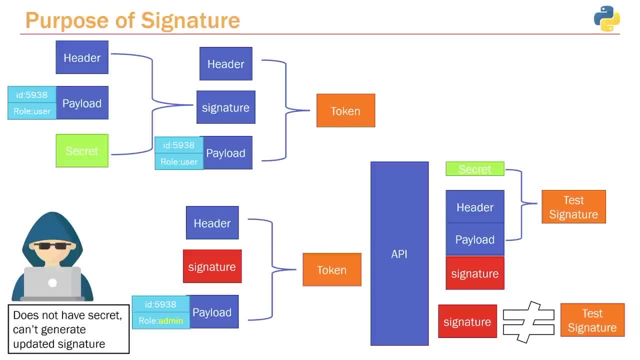 as soon as I explain this, I think you guys will see that it's not too complex of a concept. So let's break this down step by step. Let's say a user has logged into our application, he sent our credentials and our API has created the token and it's in the process of sending. 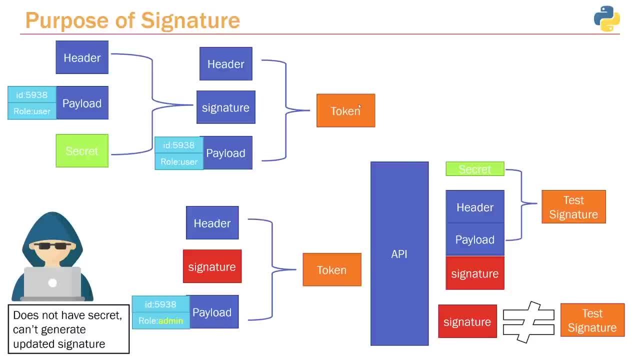 it back to the user. So this is going to be our token that we create on our API And it's going to create. it's going to have three things, the same three things we discussed in the previous slide. we've got the header, that's got all the metadata, it's got the payload right And this: 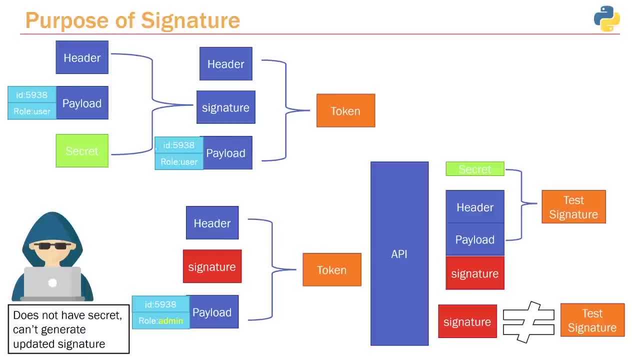 is going to have whatever information we want to put in the payload And in this case, we've decided to embed the user's ID as well as his specific role. In this case, he's a plain user. he's not like an, a special privileged user or a staff user or an admin. he's just a regular user of. 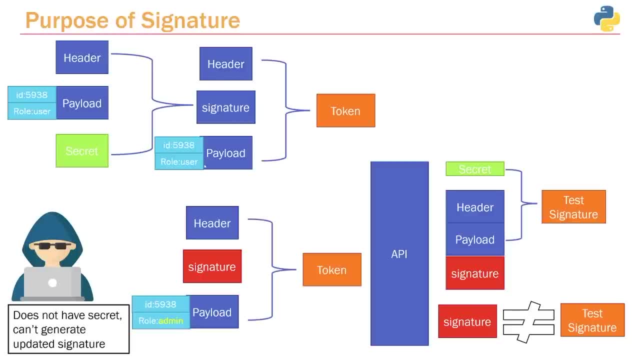 our application, So he can only do very specific things. And then we have to generate a signature, And our signature is going to be a combination of three things. it's going to be a combination of our header And, remember, this header is the same thing. So, even though our token already has, 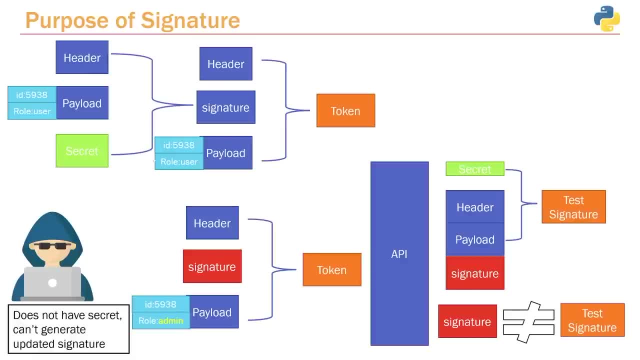 the header. what we do is we take that header, we take the payload with the specific header and we take the payload with the specific header And we take the payload with the specific pieces of information we've included in there, And then we include, finally, our special 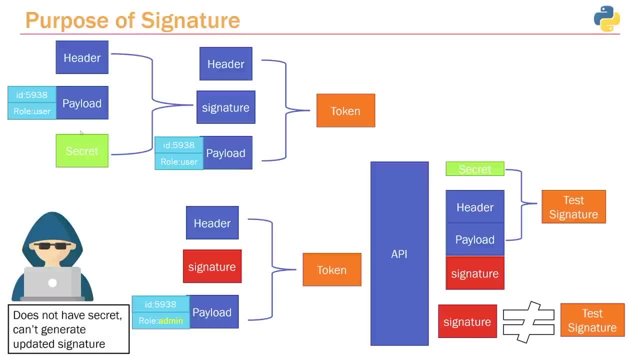 super secret password. Remember: this password only resides on our API servers. nobody else has access to it. our clients don't have access to it. the front end doesn't have access to it. only we have access to it on our API server. And this is very important because this is the special 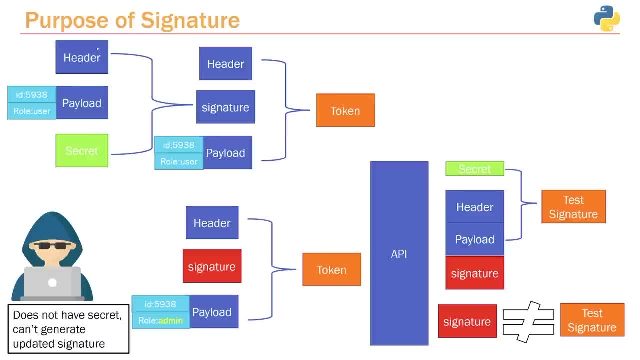 password that no one should ever have access to. And so we take all of these three things, we pass it into a hashing function, essentially, and then we create a signature, And so we take these three things and that's going to be our password, And then we take all of these three. 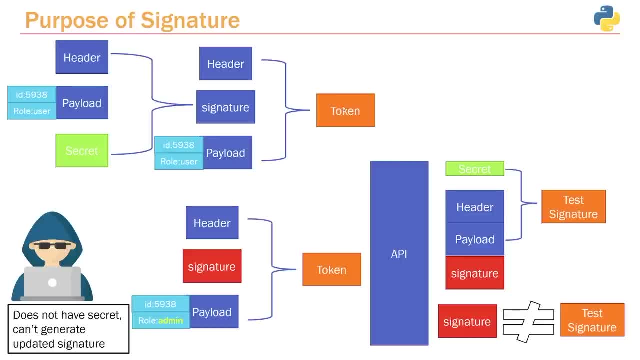 things and that's going to make up our token, And so we send that back to the user. Now let's say that we've got a user who decides that he wants to do a little bit of shady things And he wants to kind of hack our application and do some bad things to our application. 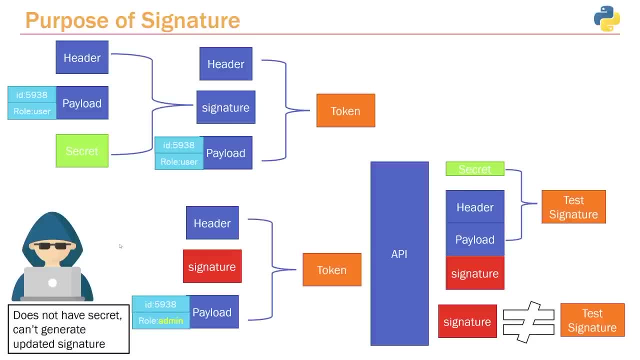 ultimately, And so what he's figured out is like: hey, look, this token, right, it's not encrypted. I can see all the data, I can see that I'm a user, And so what he's decided to do? he changed a few bits in the token to make it now read admin instead of user. 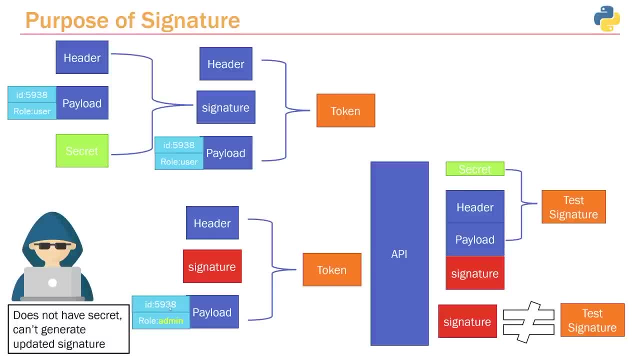 But he could have really done anything right. he could have changed the ID so that it's someone else's ID and he can potentially have access to someone else's information. It doesn't really matter. But he's changed a few things And so now he's got a this token which has the header: 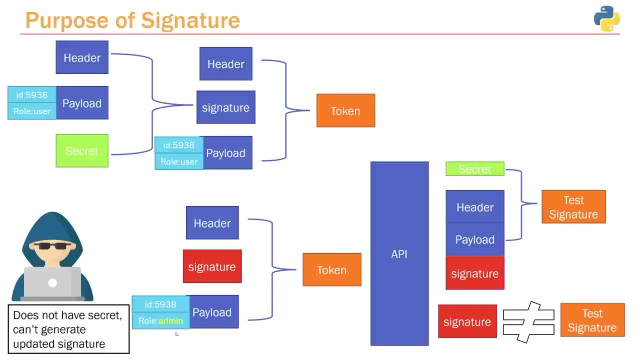 signature and payload And he's now a admin user, or the payload says he's an admin user Now, the reason he can't actually do this is because ultimately- remember- the signature that's currently in the token was generated by having a header. 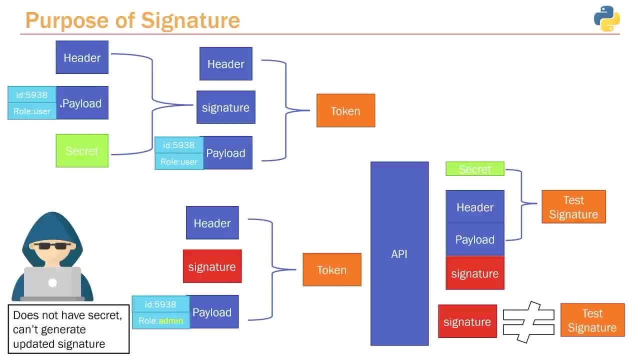 the same header and then you pass in the payload with this specific ID and a role of user And then you pass in the secret And so this signature is no longer valid. he can't use this same signature because it's not going to match up with the data that he has. So if we actually 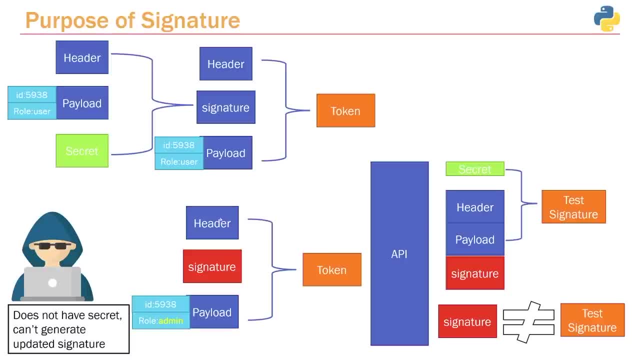 try to create a signature from this, it's going to look different, And so what he has to do is he has to create a brand new signature so that it matches the data he's sending. However, he can't create a brand new signature because he doesn't have this signature, And so he has to create a. 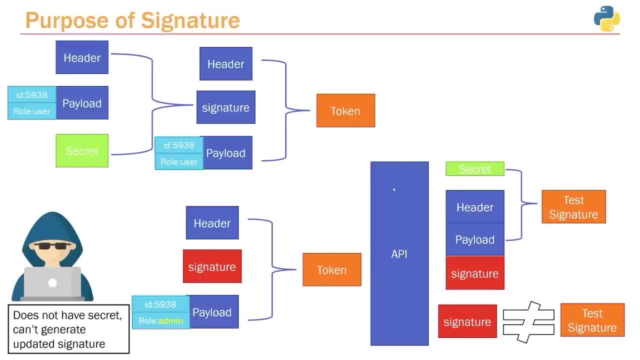 super secret special password. This only resides on our API server And so if he tries to create a brand new signature, he can only pass in the header and this payload into the hashing function to generate a new signature, And so that once again is not going to be a valid signature, because when 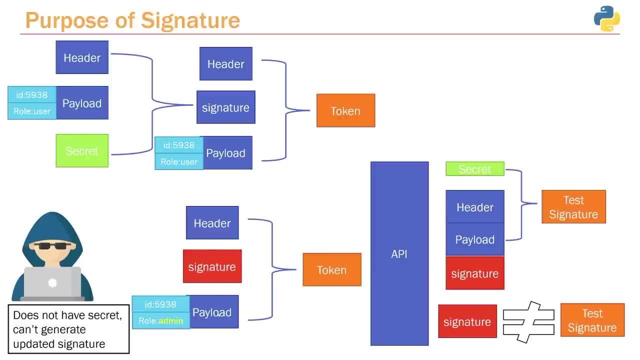 he sends, but let's say he does create that signature with only the header and the payload and no secret. what we now have, this token right, that's made up of these three things. we send it to our API And what our API is going to do is to verify if the token 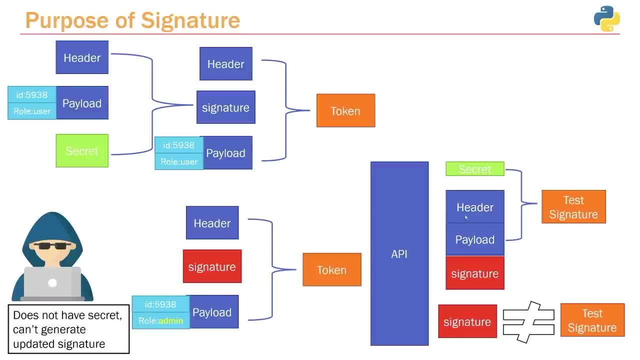 is valid. he does a super simple test: he takes the header, he takes the payload and he takes the secret And he creates a test signature. Because, remember, that's what we did in the first place, to actually create the original token: we take the header, the payload, the secret and we pass it in. 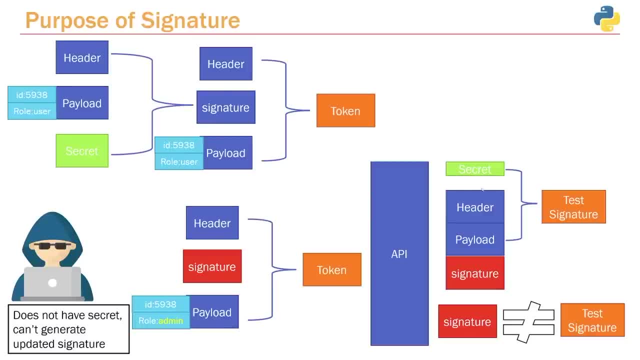 to our signing function And we pass it into our hashing function: create the signature. So we do the same thing And then we take the signature in the token that was sent by the user And we just compare them if they don't match- which they won't because, remember, he doesn't. 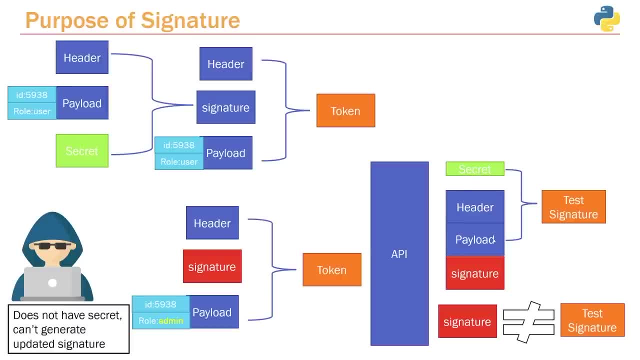 have access to the token And then we take the signature in the token that was sent by the user- secret- And since we use the secret in our hashing function, right, the signatures aren't going to match And we know that this token is not valid, So this signature once again. 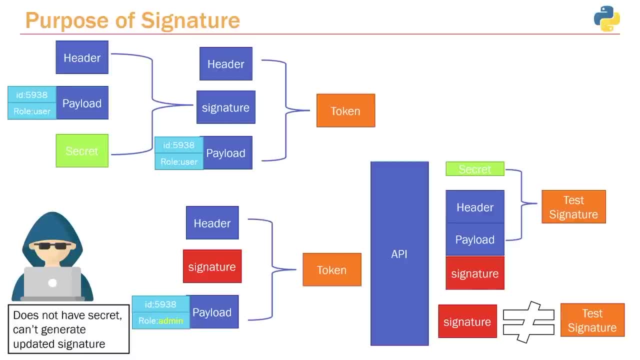 only ensures that the data integrity is still valid, that no one has tweaked any of the bits. no one's changed any of the data. that's all the signature can do. it can just verify that it hasn't been changed since we created the token in the first place. 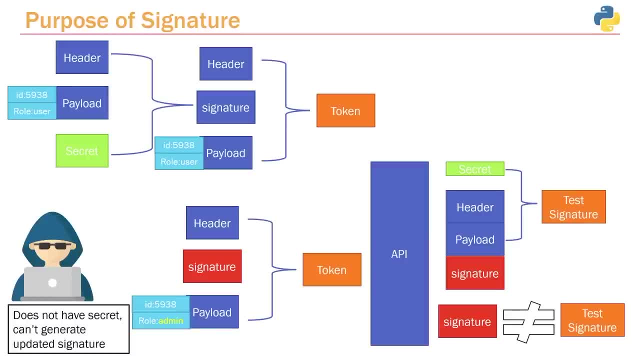 But once again- and I can't stress this enough- anybody can change the data of a token. anybody can see the data of the token. they just can't generate a brand new signature because they don't have access to the secret, And so that's why the password is so important. 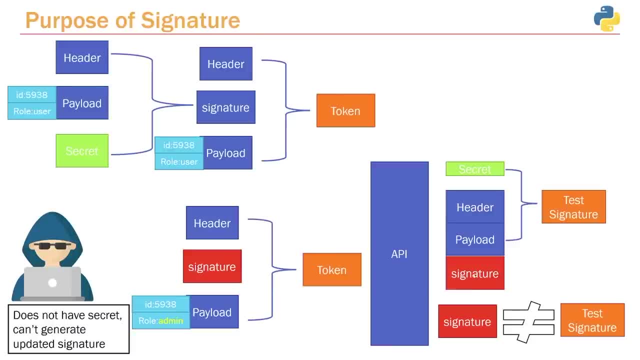 because that's how we ensure that the token hasn't been manipulated or changed in any way, shape or form. So hopefully that made sense. I didn't understand this at first. it took me a while to actually grasp why we needed the signature. I just kind of was like I'll figure. 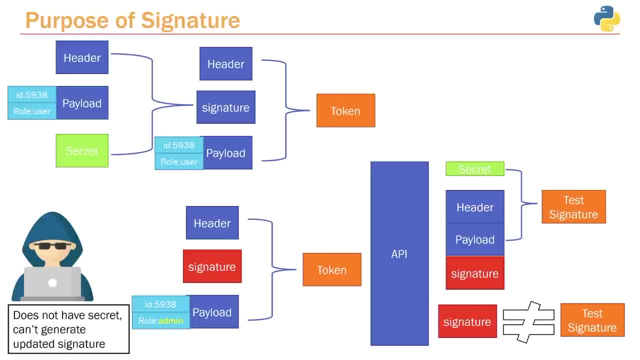 this out later. But after a year or so I was like: Oh, this is actually a super simple concept And hopefully I can do a slightly better job at it. So I'm going to go ahead and do that And I'm going. 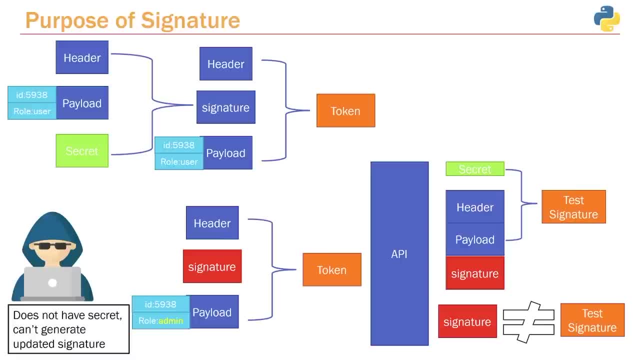 to go ahead and do that, And I'm going to go ahead and do that, And I'm going to go ahead and do that. I can do a slightly better job of explaining it than some of the documents that I read when I was first learning it, And hopefully this kind of you know gets rid of some of the unnecessary stress. 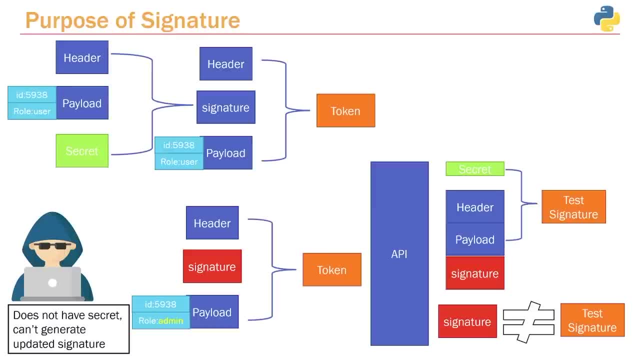 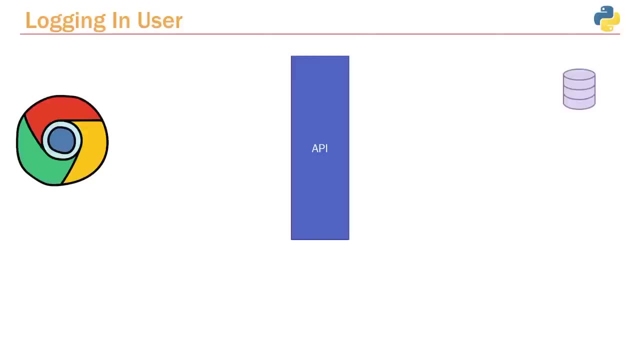 that kind of comes with learning about JWT based authentication. So once again, let's quickly take a look at how we're going to handle logging in the user. More specifically, how do we actually verify that his credentials are correct? because it's not going to be exactly the same way that you would. 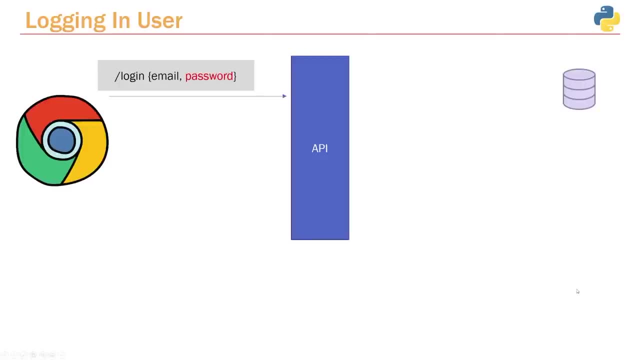 think So. the user is going to hit the login endpoint and he's going to provide the email and the password, And I've colored the word password in red because this password is going to represent what the user is trying to log in, as this is his attempted password. that's what we're going to. 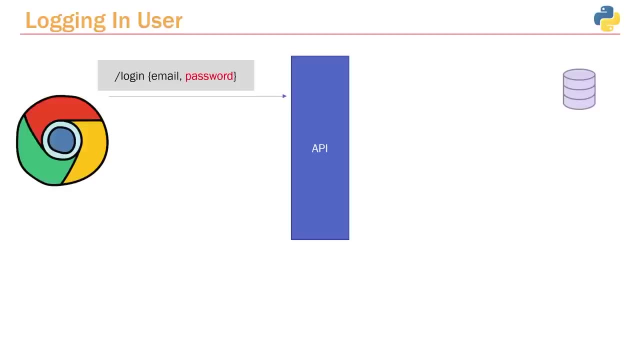 call it And that's going to be in red. And keep in mind that when he sends this password it's in plain text, right? It's just the regular password that he typed out, And so when it gets to our API. 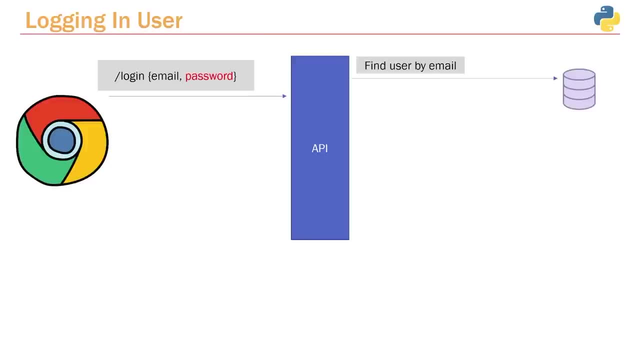 the first thing that we're going to do is we're going to hit our database to try to find the user based off his email or his username, And the database is going to send back all of the information about that user, which includes the password. However, 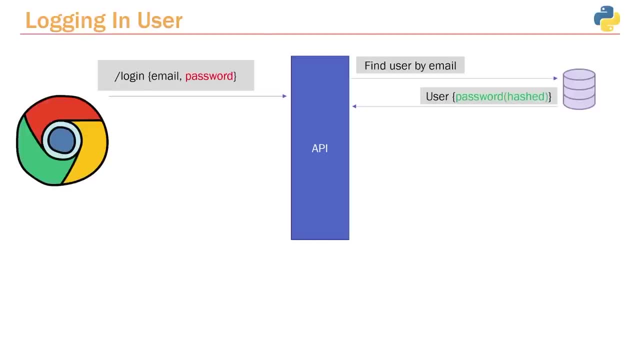 if you remember how we actually created the password and stored it in the database. we actually stored a hashed version of the password in the database so that if anyone hacks our database, the user's passwords aren't actually in plain text, so no one can really hack. 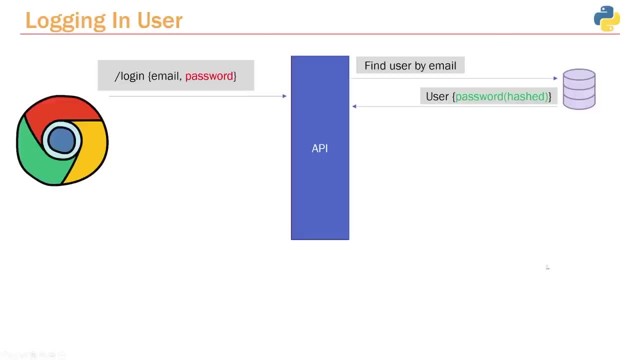 their passwords, But this creates a little bit of a problem because we have the attempted password for the login attempt in plain text. However, we've got the password in our database as a hashed password. So how exactly do we check to see that they're equal? Because right now 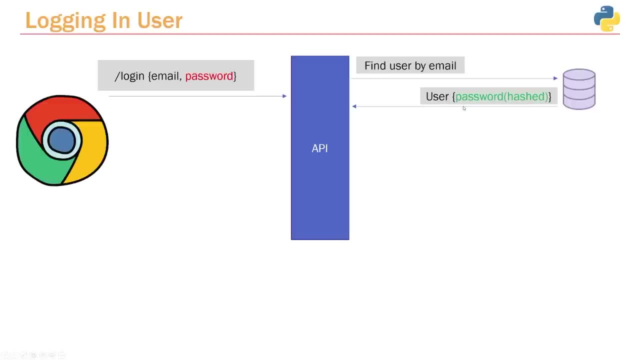 a hashed password does not equal the same as the regular password And your first instinct is to Hey, well, let's just convert this back to a plain text password. And we can't exactly do that Because, remember, a hash is only one way. So if we hash a password, we can't get the original. 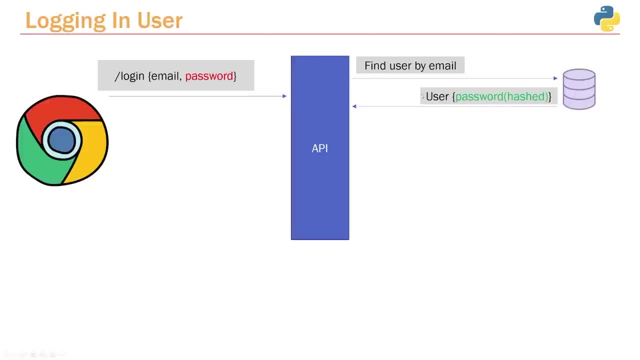 password from the hash. That's what's great about hashing a password, And if you think you can do that, that's actually what I guess, what we would refer to as encryption, but we're hashing in this case. So what do we do To verify if the passwords are actually equal? It's pretty simple: We just 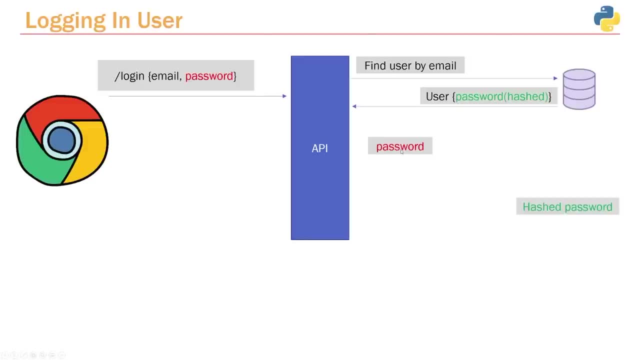 take the hashed password And then we take the raw and once again, this hash password is the correct password in our database. then we take the password attempt and we hash it again. So we hash this password And so then we get a hashed password And so if we have the correct password, 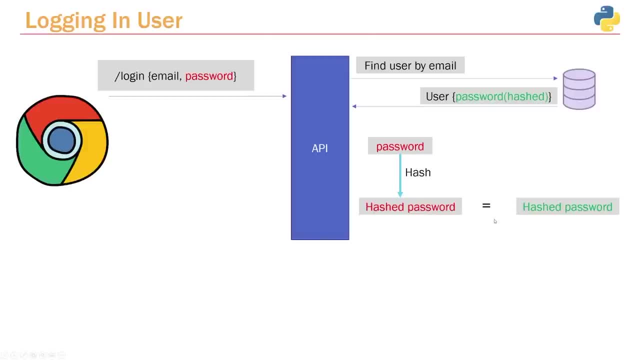 then, if we put it through the hashing function, these two should be equal, And so if they're equal, that means the password they provided us is the correct password in the database. If it's not, the, if they don't match, that means he gave us the wrong password, And so 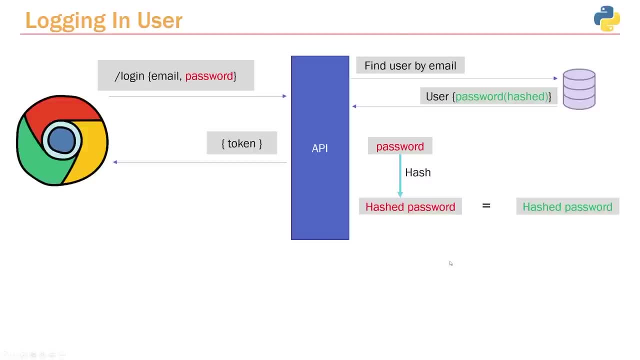 if they're correct, we'll then go ahead and send. we'll create a token first and then we'll send it to the client. So it's as simple as taking the attempted password, hashing it and then comparing it with the hashed password in the database, Because if the passwords are correct, then the 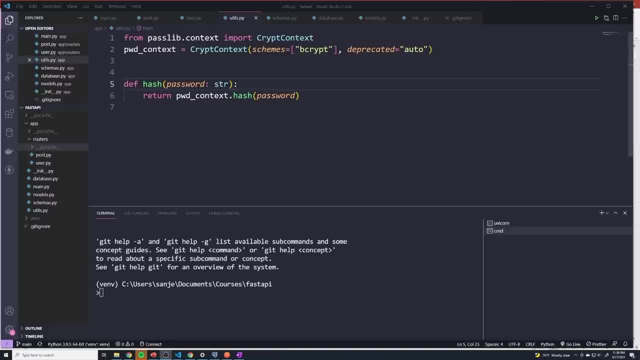 hash should be equal to hash in the database. Okay, so we're going to create the login path operation, And what I'm actually going to do is- you're probably thinking that we can just store the path operation in the userspy router. However, I think it would make more sense to 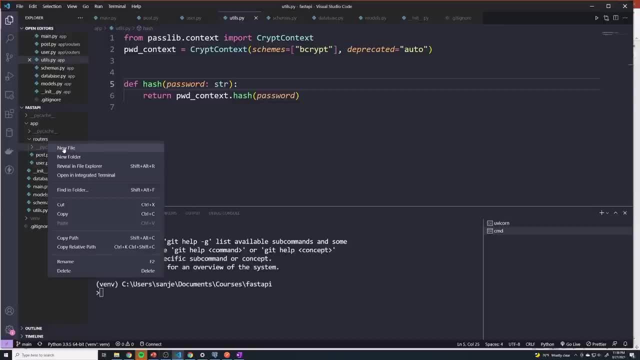 actually store this in a authentication router. So we're actually going to go ahead and create a brand new router for this, so that we can keep the user routes versus the authentication routes in two different files. However, if you really wanted to, you could store it all in one file. 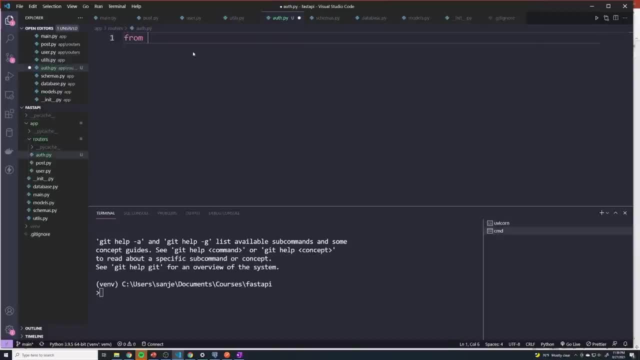 So I'm gonna call this authpy And the first thing that we have to do is, from the fast API, we're going to import a few things. we're going to import the API router, we're going to need depends, status, HTTP exception And maybe we need the response. 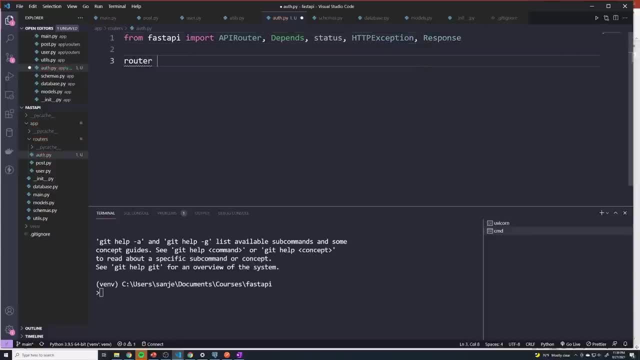 I haven't decided. And then we're going to define our router, So we'll say router equals API router, And we're going to pass in a tag, you know, just for the documentation. So we'll say tags equals authentication, All right. and then we're going to create our login, So we'll call this: 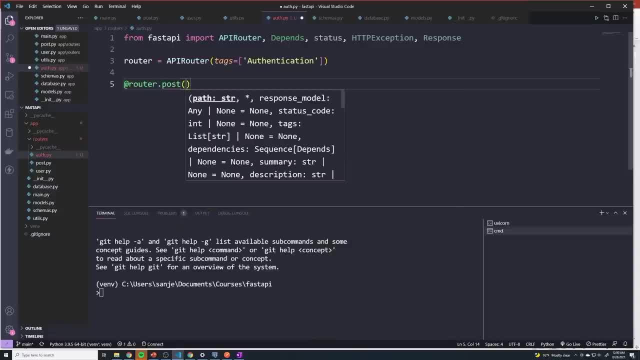 well, first of all, this is going to be a post request because, remember, the user is going to have to provide his credentials. So, generally, when you want to send data in one direction, it's going to be a post request. 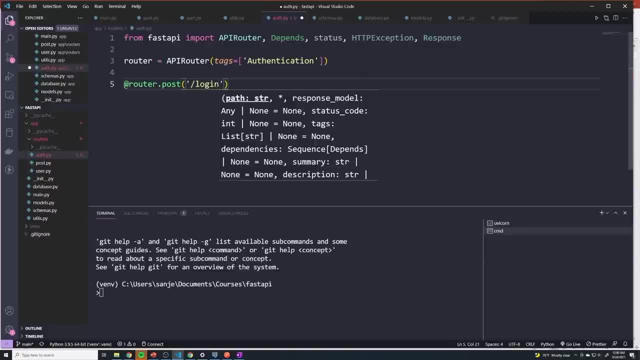 And we'll send it to the login endpoint. you can call this whatever you want. you can call it authenticate, However. I like login, And then we'll define our function And I'll just call this login as well, And because we're ultimately going to have to fetch the user from the database. 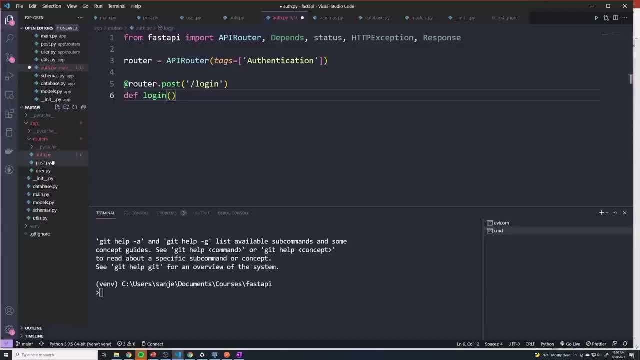 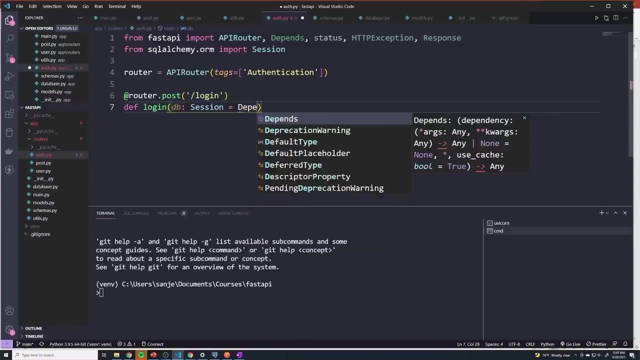 we're going to have to import our, our database session, And so from SQL alchemy we'll say dot or m import session, And so we'll do the same thing that we did with every other path operation. I'll say DB session equals, depends, And then we're going to have to actually 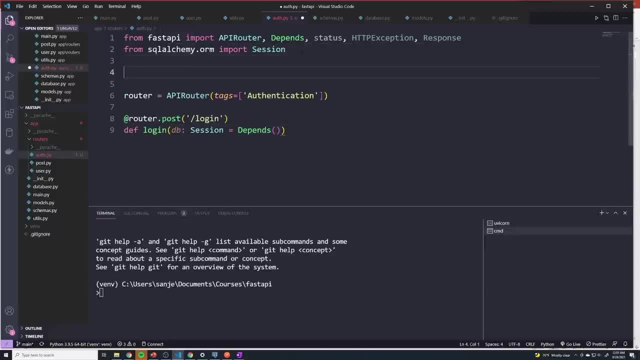 import our get DB function. So from here we'll do from, and we have to go up a directory and I'll say database import session. sorry, not session. Actually, you know what I'm gonna do, I'm just 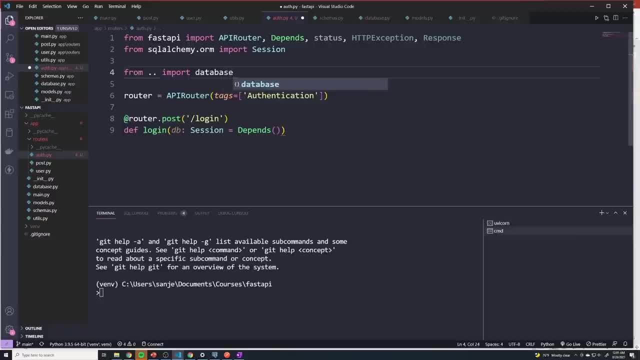 gonna say from dot, dot import database, And then I can just reference it as database, dot get underscore DB. And since the user is going to be providing the login information, I think it makes sense to set up a schema so that we can ensure that they provide the exact pieces of. 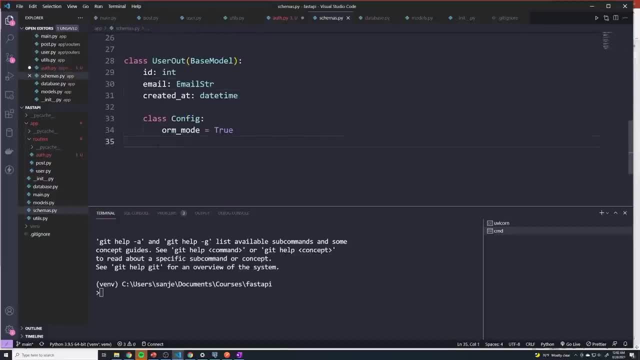 data that we ultimately want, And what we're going to do is we're just going to create a new class And I'm going to call this user login, And this will extend the base model, as usual, And the two pieces of information that we want: our email. 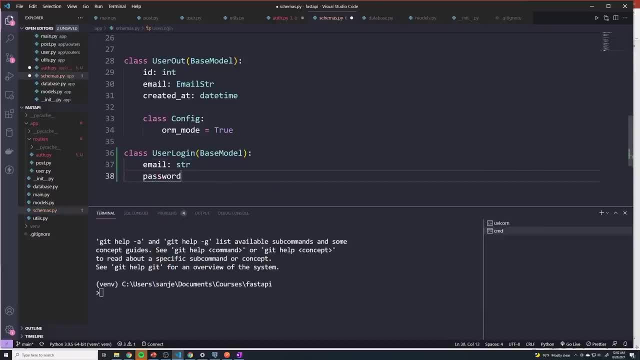 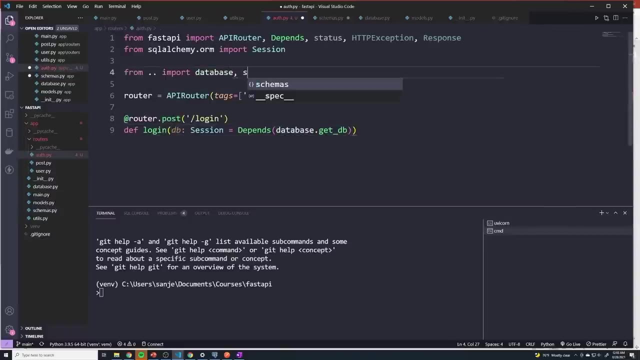 which is going to be a string, and then we can do password, which is going to be a string. Actually, I'm going to, I'm going to use an email string, like we did before, And then, from our author, P Dom, also going to import schemas, and here I'm going to store the 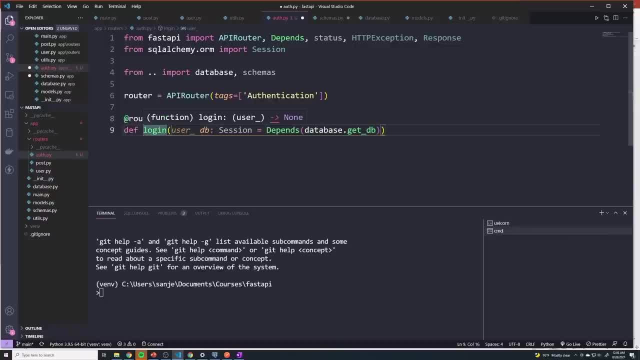 schema as a user credentials is gonna be schemas that user login. All right, and so now we can access all the user information, or the attempted login information with the user credentials variable And we're going to make a request to our database, specifically our DIY load. This is going: 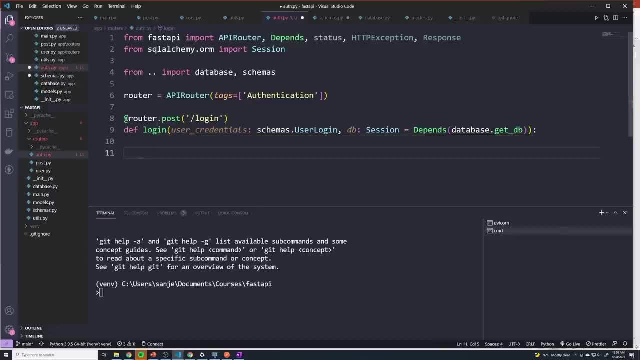 to give us the新 skill. We're going to give it a string And we're going to discuss a little bit about that. our users table to retrieve the user based off of his email. So we'll say DB dot query And we'll 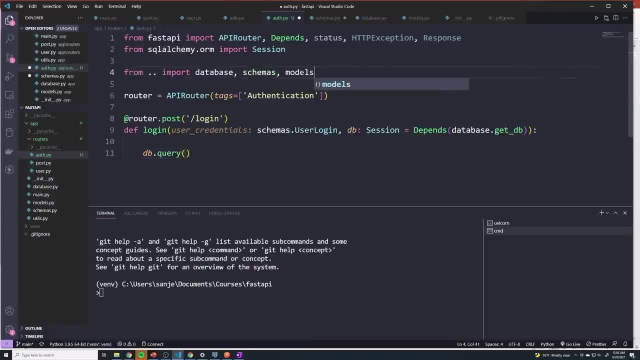 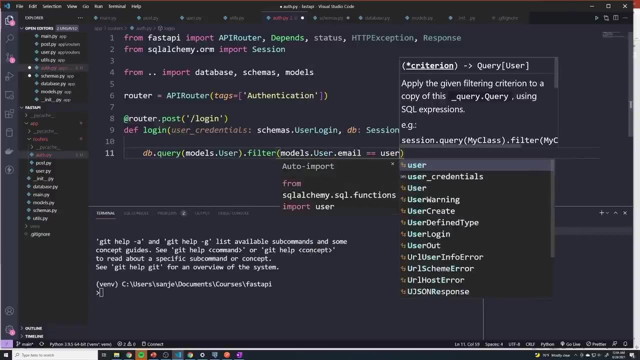 and we have to import models. now that we can access it, We'll say models dot user And then we have to filter based off of the email. I'll say models dot user. once again, dot email equals, equals, user underscore, credentials, dot email. And then there's only going to be one user with that. 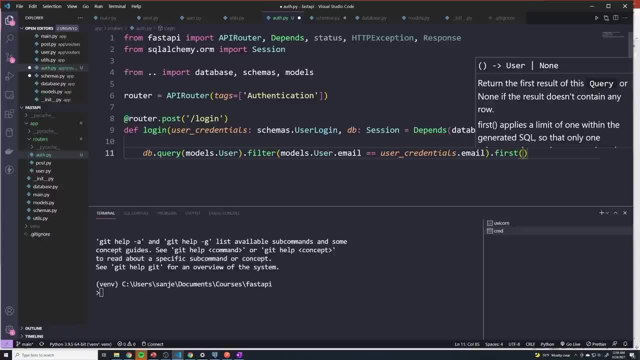 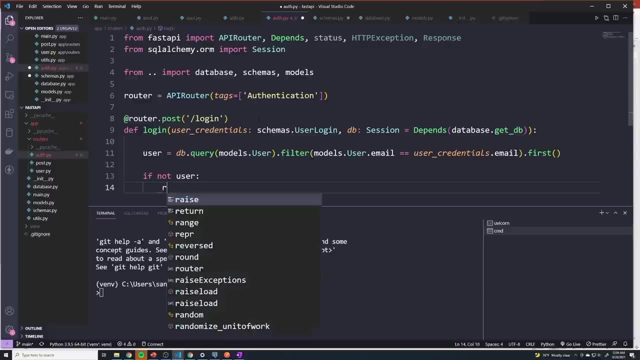 specific email. So we'll do first And we'll store this result in a variable called user. Now, if there's no user with that specific email, that we're going to return a error or we're going to raise an exception. So we'll say: if not user, we're going to raise an HTTP exception And the status: 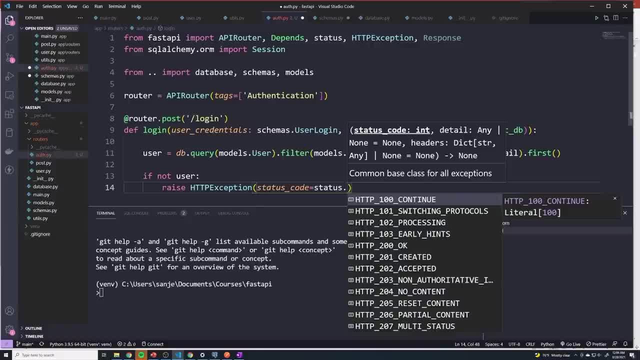 code is going to be user And we're going to say: if not user, we're going to raise an HTTP exception. The code is going to be status dot and I'm trying to remember what code will. it's going to be a 404. 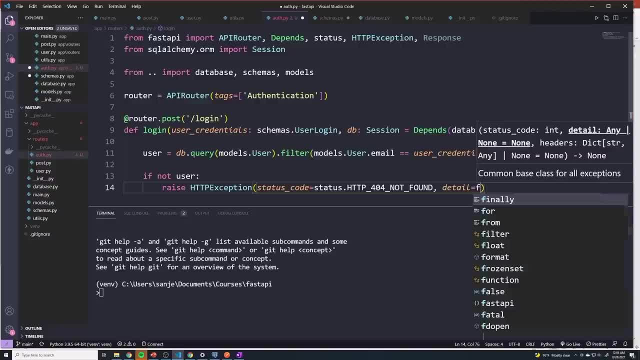 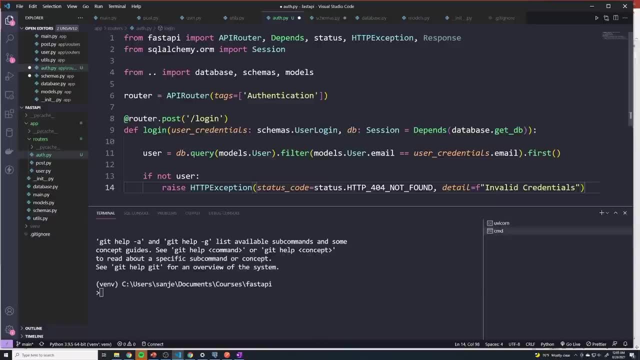 because that user doesn't exist. And then the detail field: we're just going to say invalid credentials, Because normally with authentication you don't want to say, hey, this is the wrong email or this is the wrong password, because you don't want to make it a little bit easier for them. 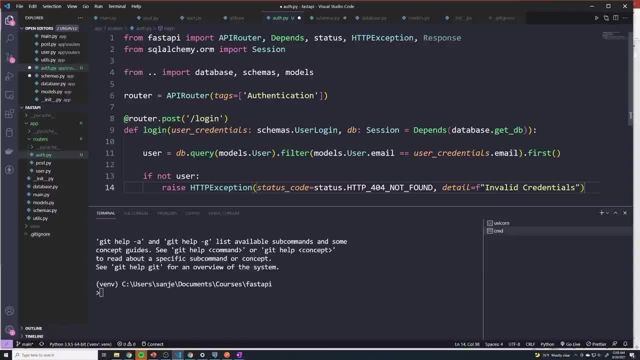 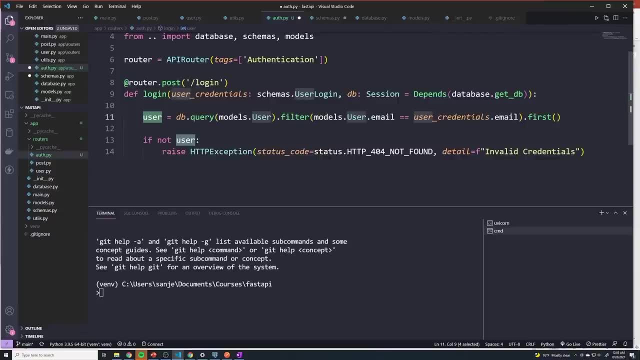 to kind of guess other people's information, Just say this is invalid credentials. let them figure out whether it's the email or the password. And then after this, once we verify that we did actually get a user object, we have to verify that the passwords are equal. So this would be, you know, performing that logic of of. 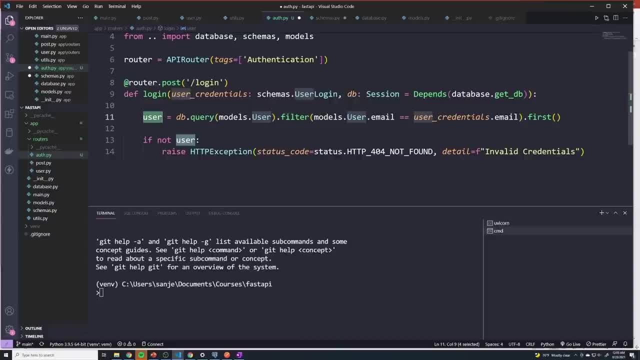 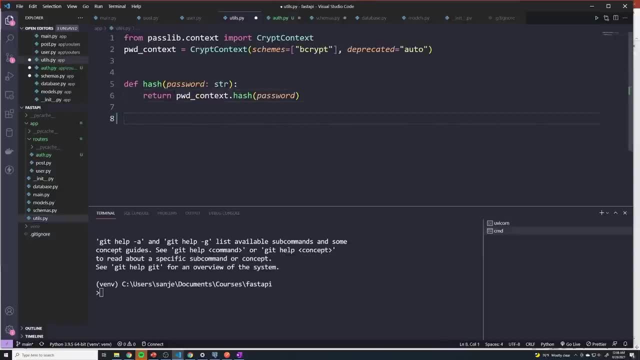 hashing the password that they gave us and seeing if that it compares to the password from the database. And so what we're going to do is we're going to create a new function in the utils folder that's going to be responsible for comparing the two hashes, Or actually it's going to take in the 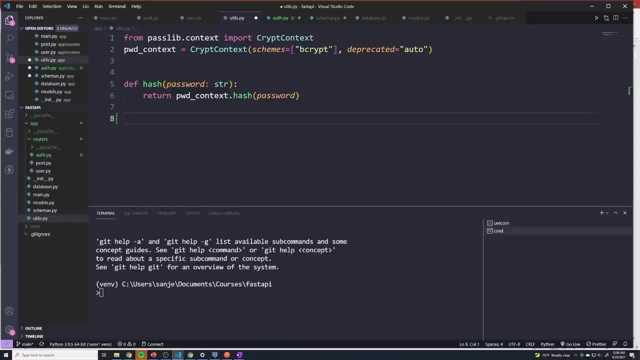 raw password, the password attempt. it's going to hash it for us and then it's going to compare it to the hash in the database. So we'll create a function, we'll call it a verify, And it's going to include the plain password, which is the password, And then it's going to compare it to the 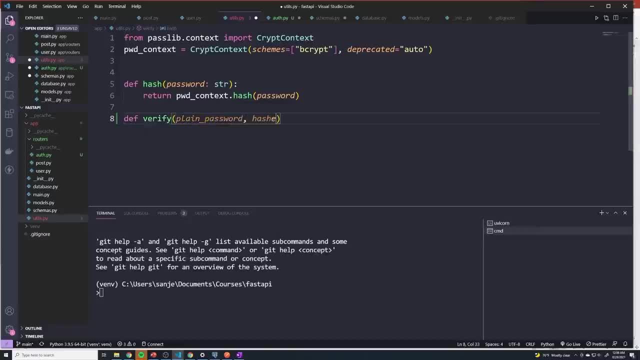 password the user is trying to attempt, And then the hash password which comes from the database, And all we have to do is just return And then we can reference the PW context right. So if you want to hash a password, you just call the dash, the dot hash method. However, it's also got a nother. 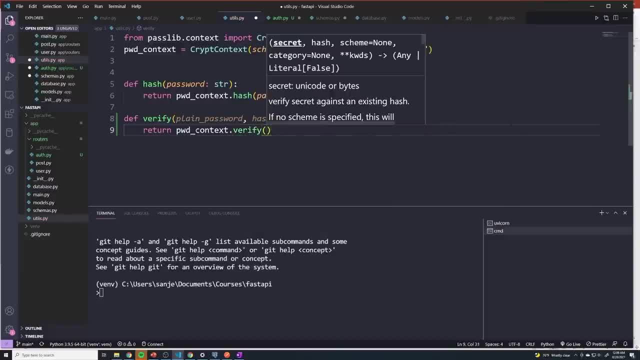 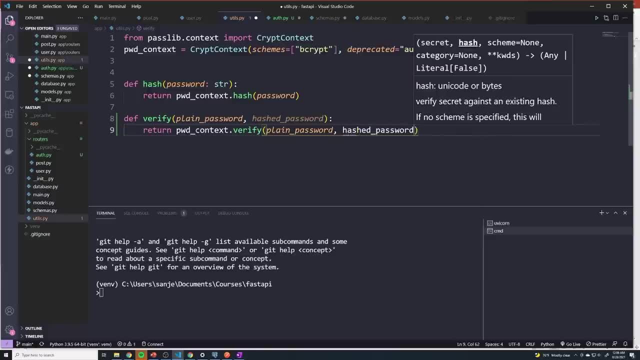 method for us which is verify, So it's going to perform all this logic for us. So we just pass in the plain password And then we pass in the hashed password And it's going to figure out the rest. Now you're thinking, well? 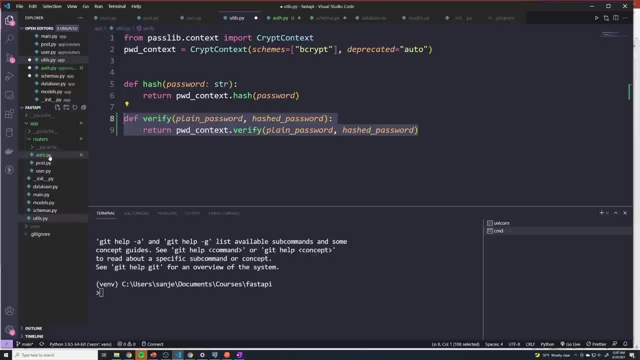 what is the point of such a tiny function? Why don't we just include it in our authpy? Well, we 100% could, because you know it's it's really two lines of code. it doesn't really make sense to. 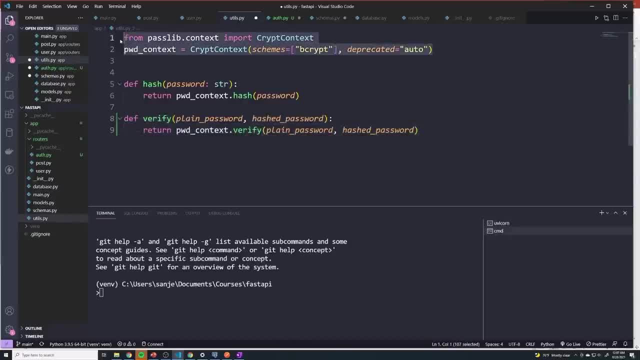 store it in another file. However, then we also have to import all of the the bcrypt code, And I like to have everything kind of separate. So keeping all of the bcrypt logic in one file just makes things a little bit easier to manage. But in our auth folder we can import utils now. 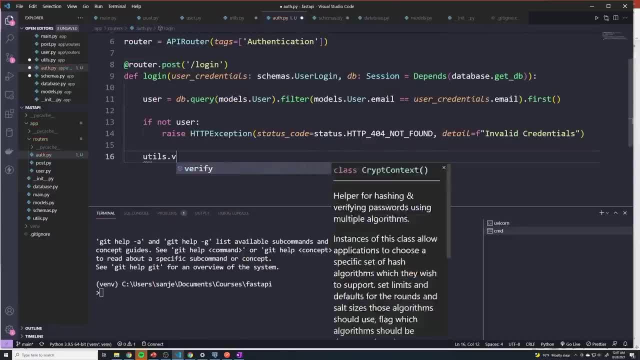 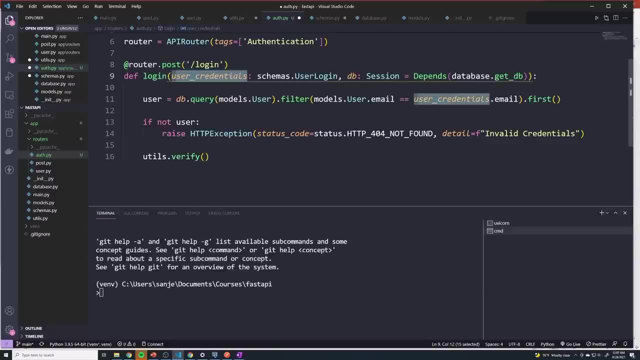 And we're going to run the utils dot verify And we're going to pass in the first the plain password which is going to be stored in user credentials. So we'll say user credentials, dot password And then we pass in the hashed password. 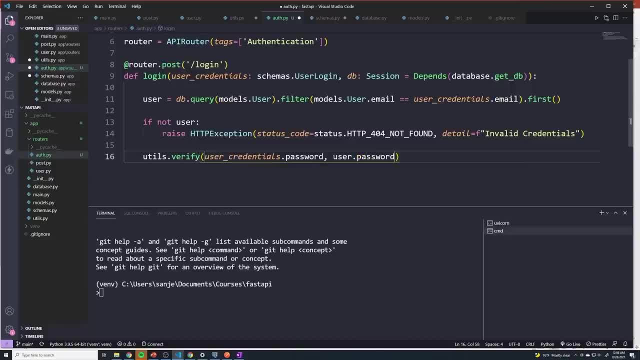 from the database which is stored under users, we'll say user dot password, All right, and if they are not equal- so if they do not equal each other, which means they provided us the incorrect password- then we're going to raise another HTTP exception. 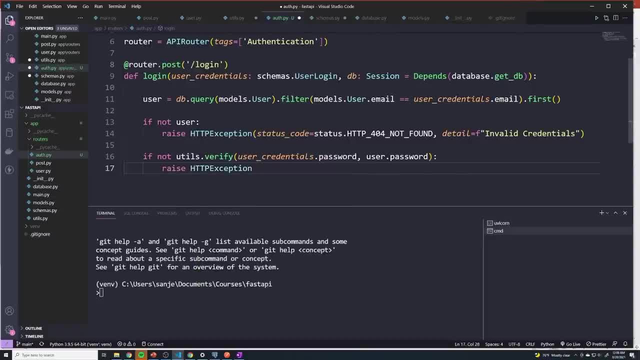 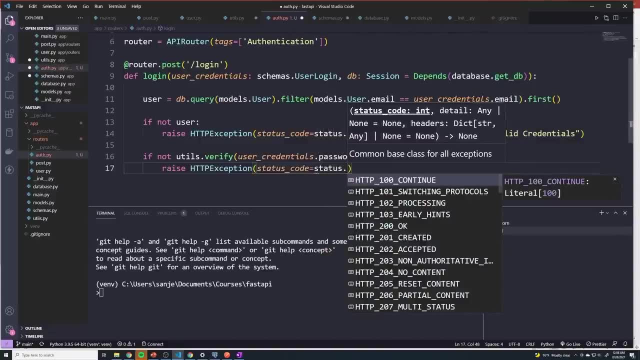 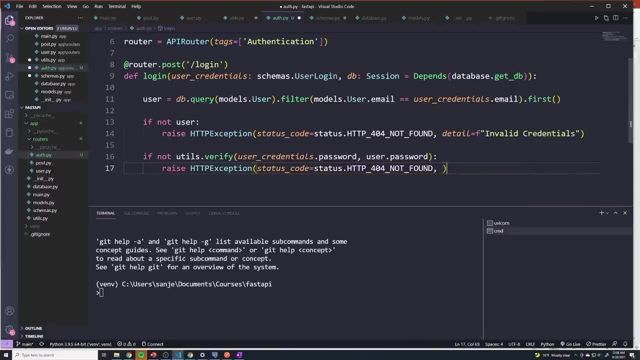 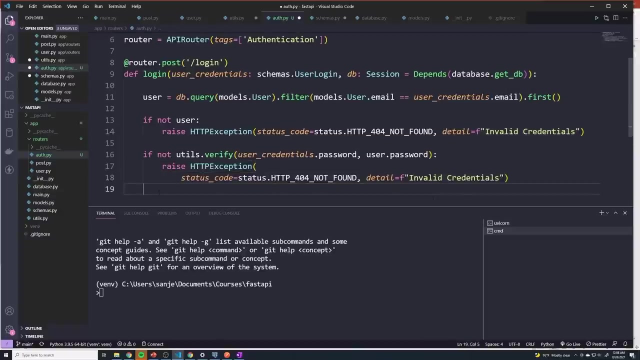 And this is going to be the same thing. we're going to send a status code of 404.. And the detail is going to be the same thing. we're not going to tell them that it was the wrong password. we're just going to say invalid credentials, so that it's not easy for them to 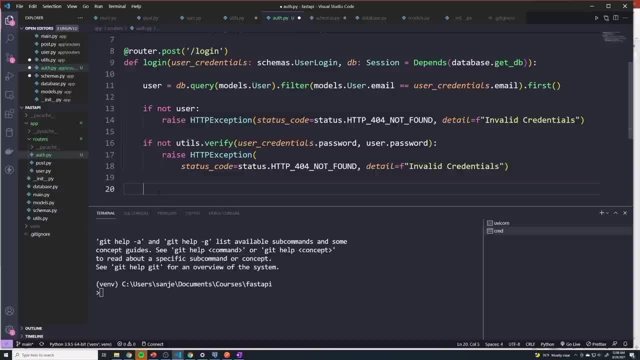 kind of keep guessing passwords or emails, All right, And then at this point what we would do is we would create a token- which you know, we haven't really gone over how to do that- And then we would just return- return token. 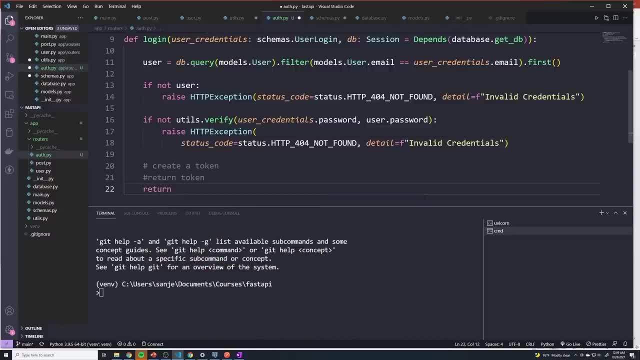 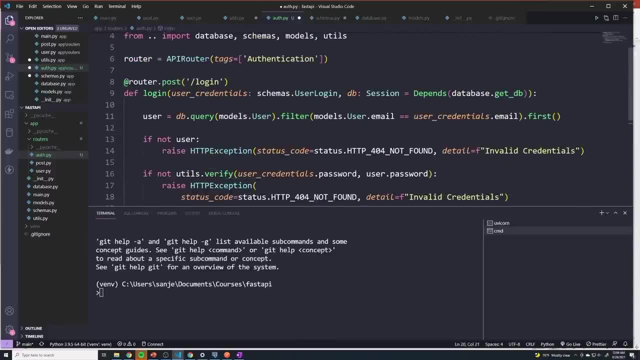 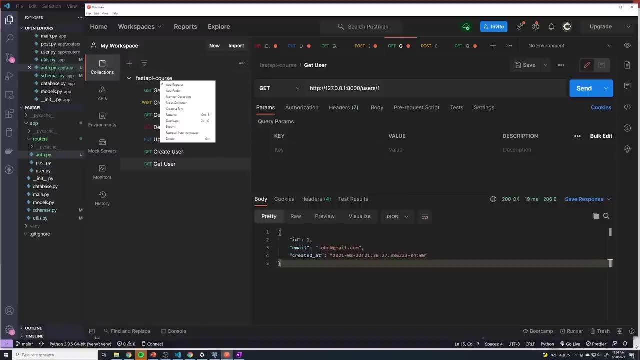 But once again we haven't done that. So I'm just going to return And we'll just say token. And I'm just gonna say example: token. right, because we haven't implemented that logic. But I do want to make sure that the rest of the code looks good. So we'll try that out And I'm going to go in. be it a. 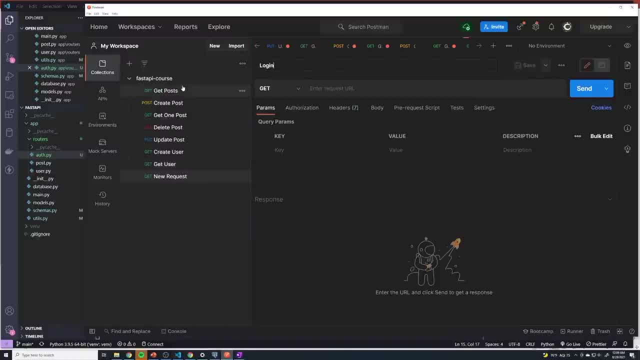 new request. This will be login user. be a post request. Copy this. Actually, this is just going to be slash login And then in our body we're going to provide some JSON And here we're just going to say: email is whatever And password is whatever. 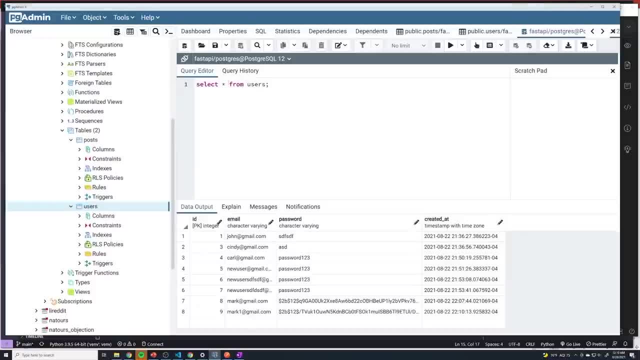 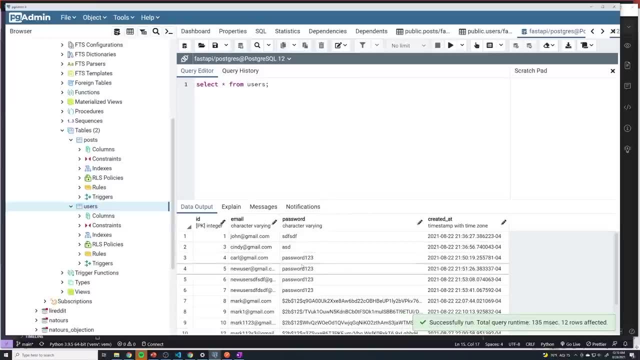 And before I actually do anything, I'm going to run a query on my database Because, if you see, I've got a couple of users that don't have hashed passwords. So I'm actually going to delete everything, just so I can clean up some mess. And I'll just say: and what I'm actually. 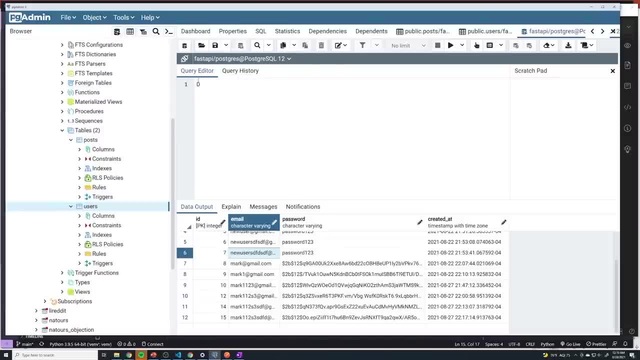 going to do is I'm just gonna delete everything. I think that's going to just make things simple, because I don't even remember these guys's passwords. So it's going to create some issues for us. So we'll just say: delete from, And then I'm going to go ahead and delete everything And 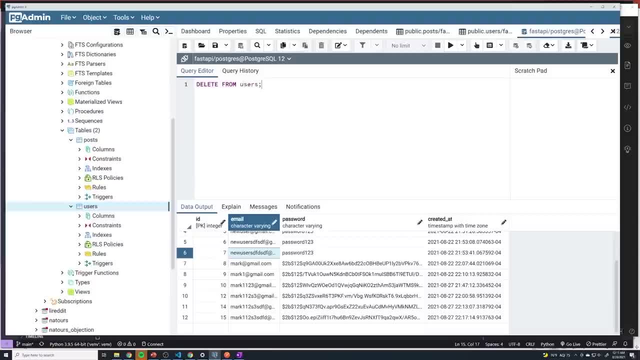 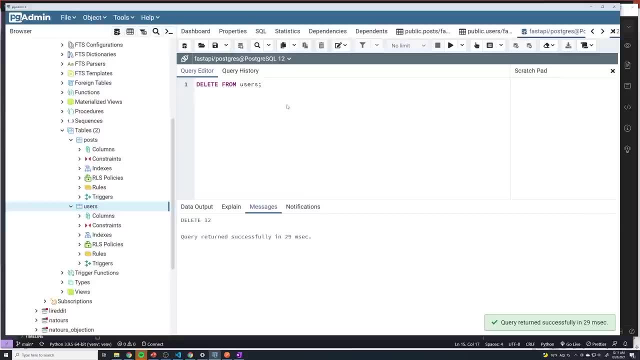 I'll say users and then I just won't provide any condition. So this should delete everything. We'll run that And you can see that it looks like it deleted all 12 results And that's perfectly okay And I'll add my original query back: select star from users And we're going to. 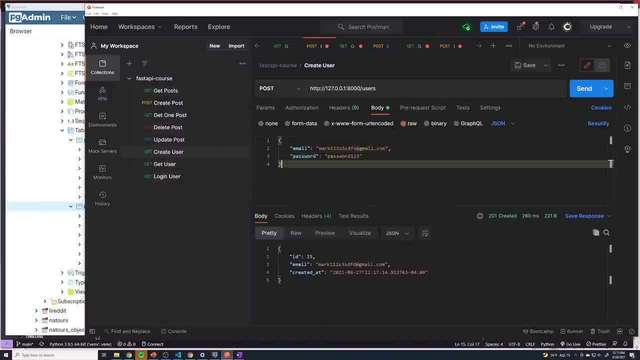 do is we're going to just register a new user. So I'll do create user And I'm going to call this Sanjeev at Gmail And then the password is gonna be password 123.. Let's create that user. Let's take a look. Alright, we've created that user And now let's log in this user. So we'll go. 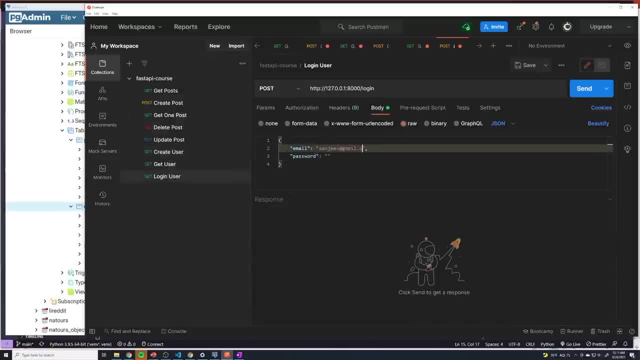 to login and I'm going to provide my Sanjeev at Gmail And then we're going to provide a password, which was password 123.. Let's try this out And it looks like we ran into an issue. So what Well? 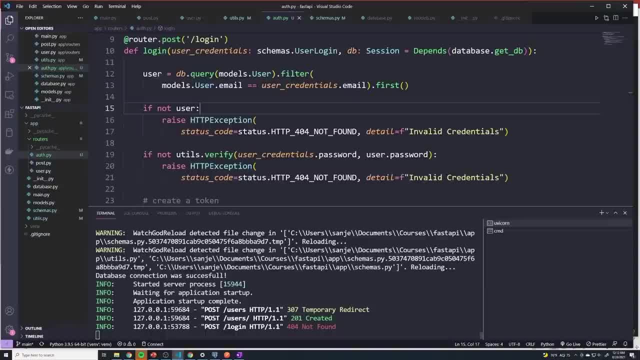 first of all, that's the wrong error message. I'm not sure why it gave me that. Let's just, it should say invalid credentials. So where is this? I don't know, I don't know, I don't know. 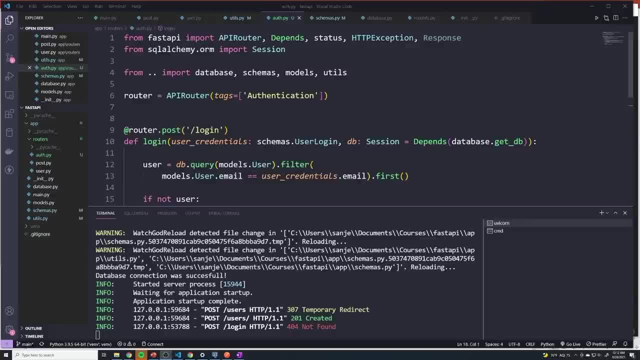 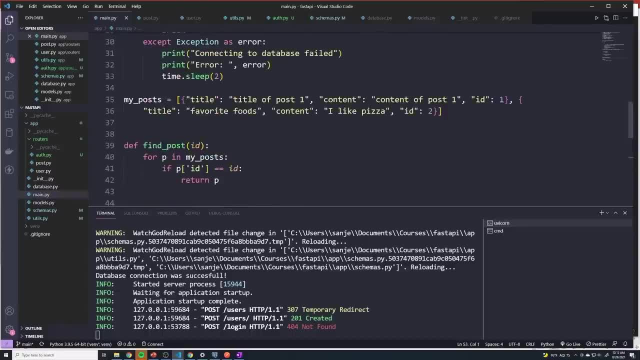 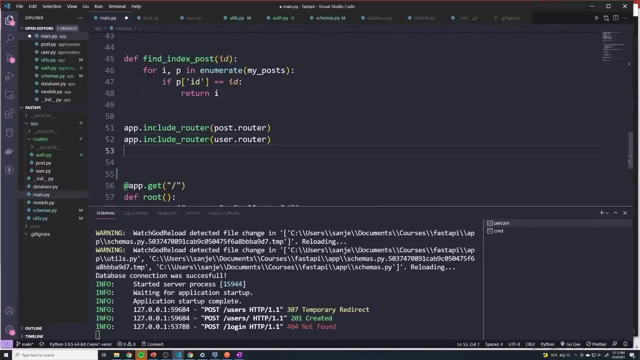 It's actually happening. And, guys, I made an absolute silly and stupid mistake. I forgot to actually wire up this router in our main dot p y file, So it doesn't even know about it. So let's import this. We're going to say import auth And all we have to do is just one skin And I'm just. 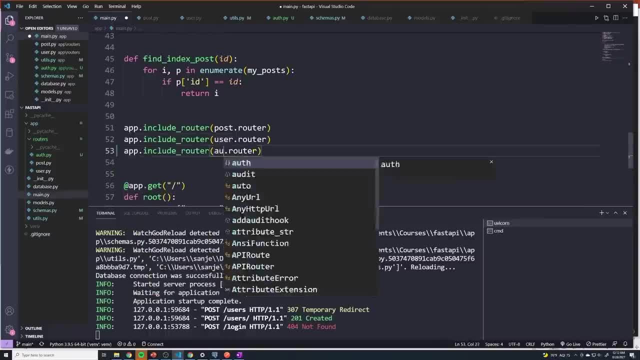 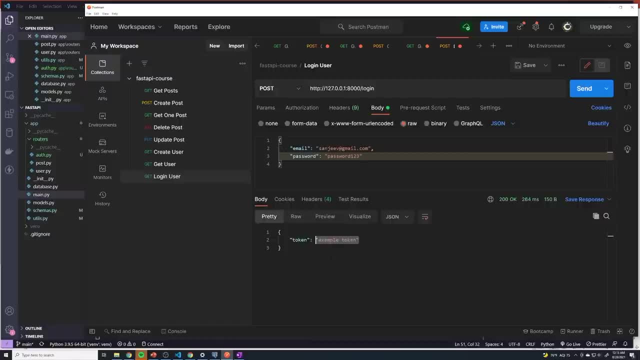 going to copy this And we'll just say: auth, dot, router, Alright, let's try this again. And we've got our example token, which means that we verified that the passwords are correct and everything was good to go. We just haven't. 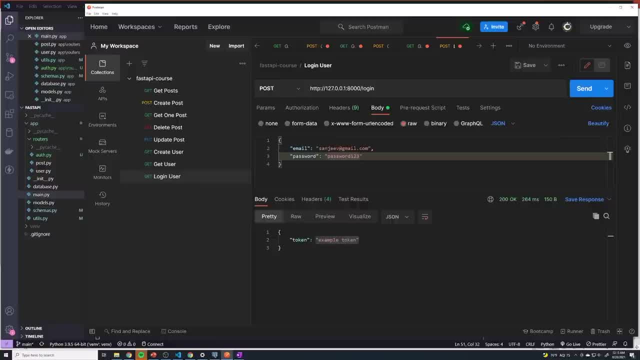 implemented the logic for the token, But let's just make sure that when we put in the wrong password, it still works, Or actually it shouldn't work And we get invalid credentials. Let's put the right password back in And then let's use the wrong email. 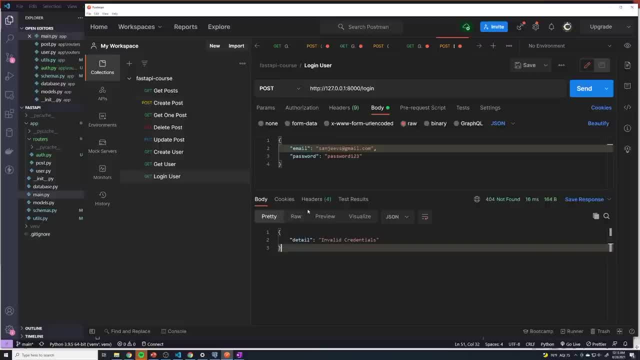 And we get invalid credentials as well. So so far we are almost done with the whole login process. The next thing that we got to do is handle creating a token. it's not going to be the default, But I do want to save that for the next video. Now, if we head on over to the fast API, 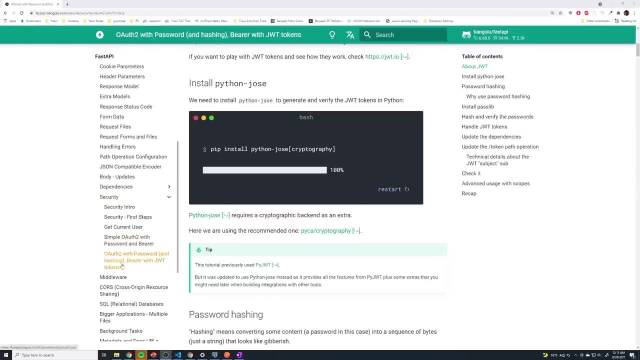 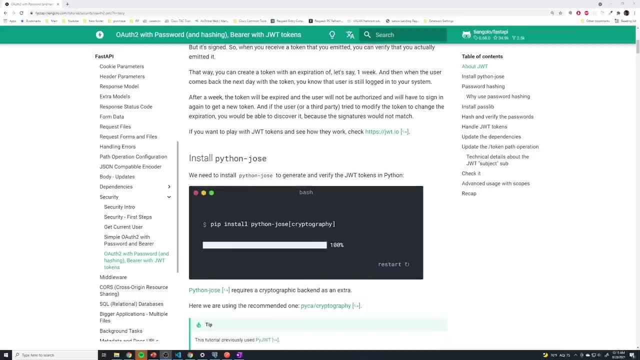 documentation under security. there's going to be oh wash with password, And so most of the things that I cover are going to be coming from this documentation right here. Now the first thing that we have to do is we have to install a library that handles signing and verifying JWT tokens And 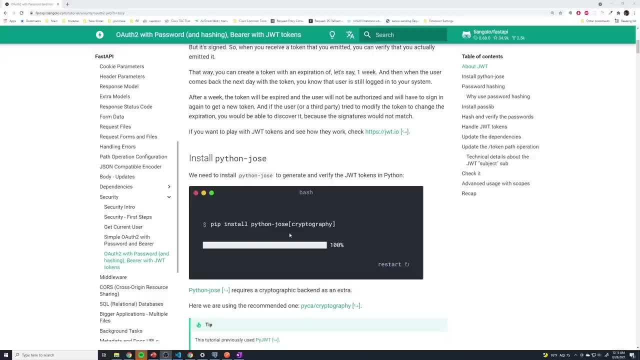 so we're going to use this Python, dash and Josie library and then we have to provide a cryptography back back end. So we're just going to copy this line right here And we're going to write a0, you, let's do that in this first line right here, And it's just going to write an extract from each of. 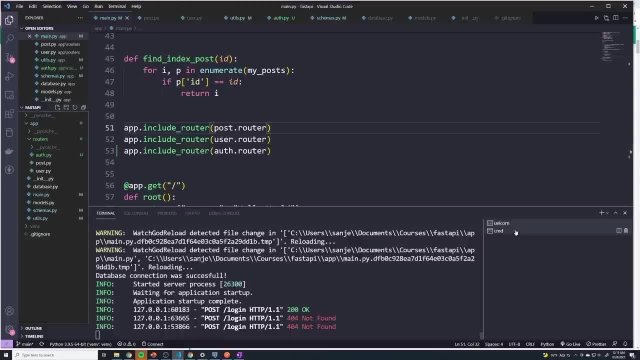 these entries of the go to code, but not the qualquer Babeş крайćim dificult, as well as the buttom line right here, And we're going to run this in the command line. And what I'm going to do is when: 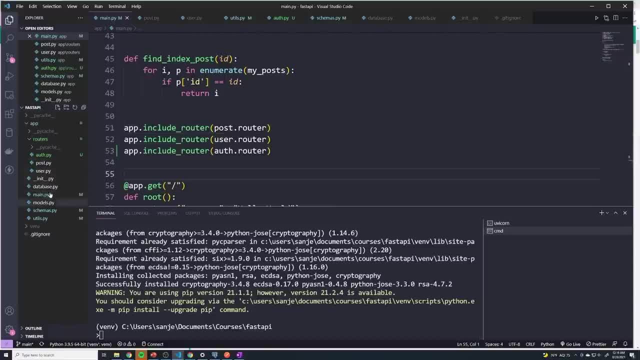 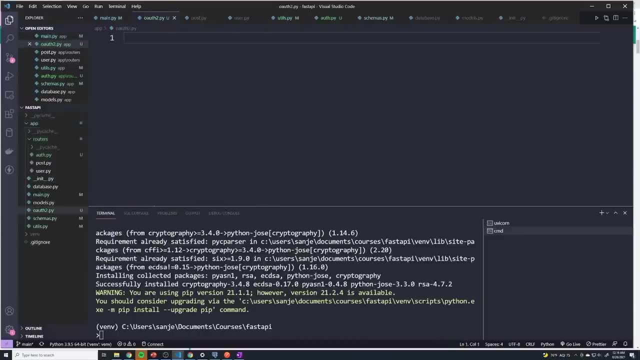 it comes to authentication and anything with JWT tokens. I'm going to create a new file And I'm going to call this OAuth two, dot, py, Alright, and the first thing that we're going to do is we're going to import from Josie. we're going to import JWT, error and JWT. Now there's going to be three. 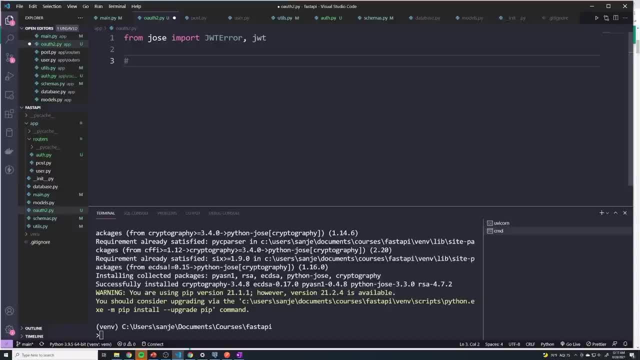 things, three pieces of information for our token. Well, actually, well, there's three pieces of information, But there's three other things about the token that we need to provide. So we're going to say we're going to need the secret key. right, That's that special key that I mentioned, that 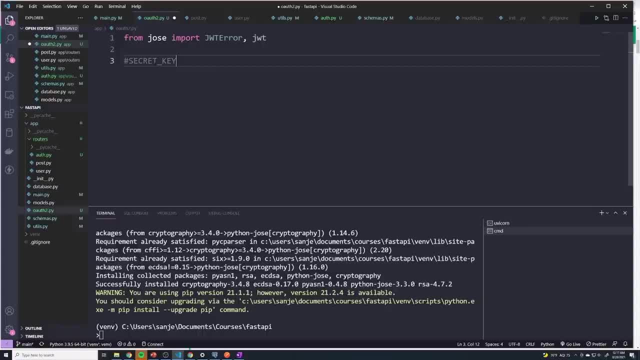 ultimately handles verifying the data integrity of our token, which resides on our server only. So we're gonna have to provide that secret key. we're also going to need to provide the algorithm that we want to use. We're going to be using HS 256.. And then we're going to need to provide one other thing, which is: 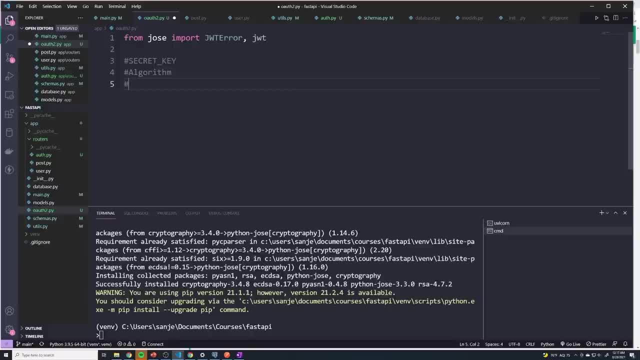 the expiration time of the token. So we haven't really discussed the expiration time. if we just give a plain token without an expiration date, that means that users logged in forever And there's no application that just lets a user log in forever. I don't think. 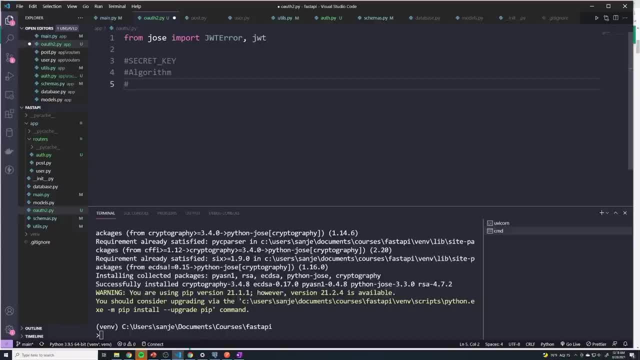 So we're going to provide a expiration time so that we can dictate exactly how long a user should be logged in after they actually perform a login operation, And so we need an expiration time. And what we're gonna do is I'm going to just save these as variables, I'm gonna say secret key. 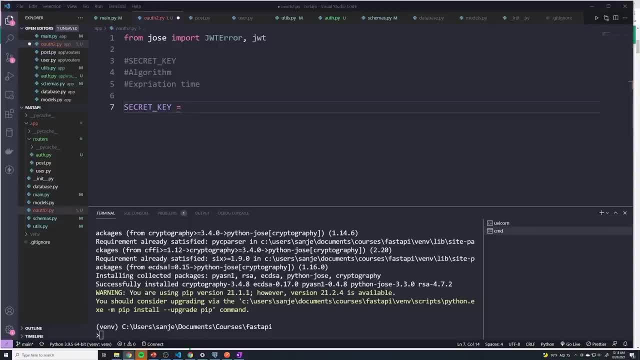 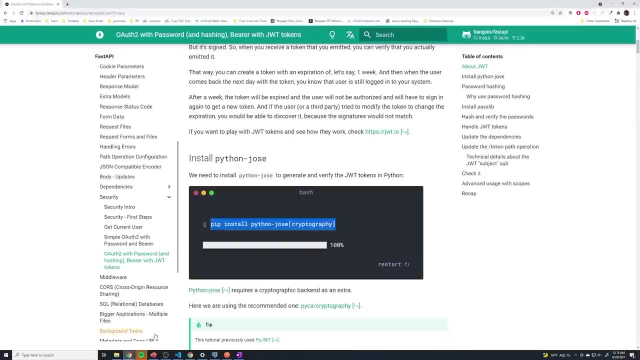 equals, and then this is just going to be some arbitrary long text. I'm just gonna paste that in here And if you're just wondering why I mean this, if you just want to just follow the documentation, actually you'll see that they do the same thing, So we just need to. 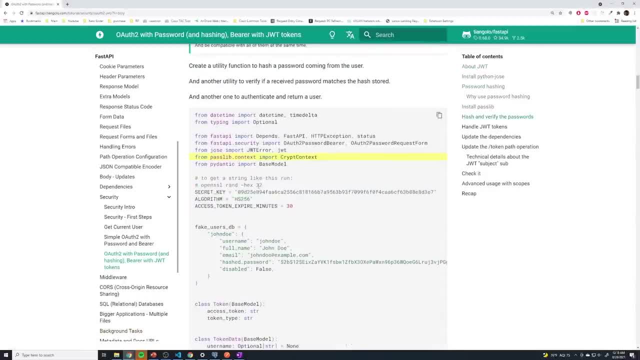 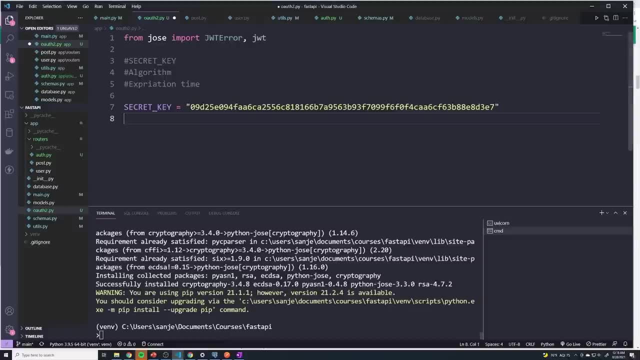 give it some really long text in this case, And it even gives you a command to kind of get a string like that for your password, Because you you could theoretically just put: you know hello or something here, and that's going to work just fine. However, it's not quite as secure, But 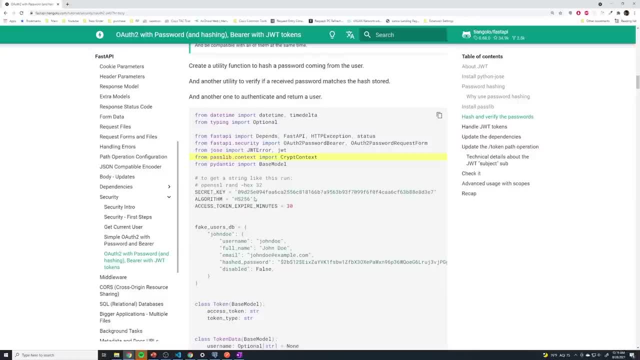 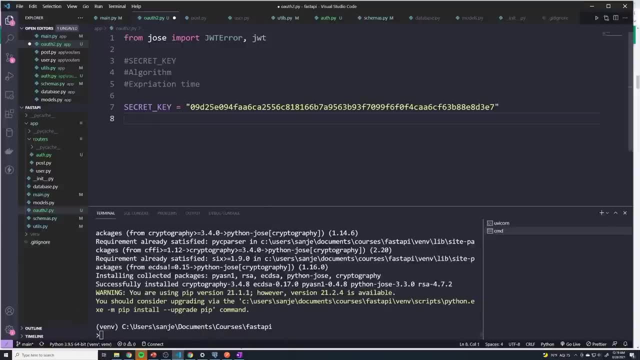 for learning purposes, it doesn't matter. just provide some kind of string, right, And then the algorithm is going to look like this, And then the expiration time is gonna look like this. So I'm just going to copy this from the documentation And then we're going to define our function. So 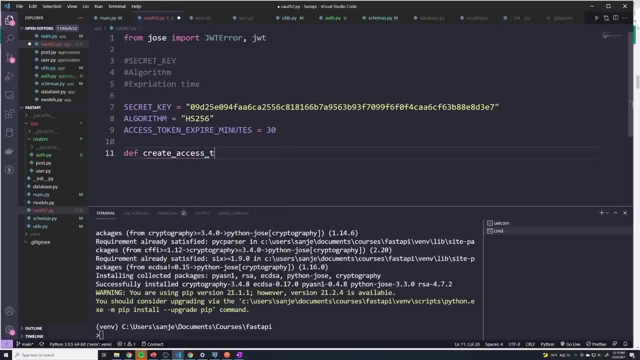 this is going to be create access token And what we're going to do is remember the access token is going to have a payload. So whatever data we want to encode into the token, we have to provide that. So I'm going to pass it in as a variable called data And this is going 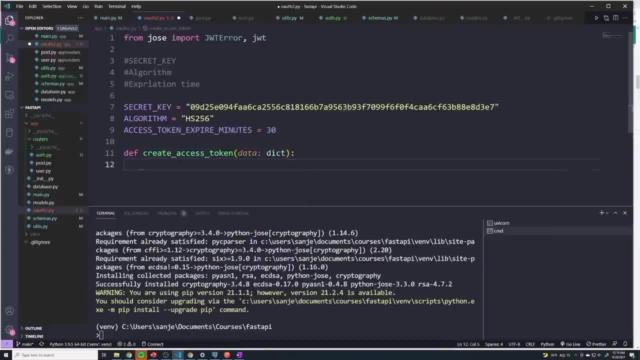 to be of type dict, And what we're going to do is we're actually going to make a copy of this data because I don't want to actually change it. I want to make a copy of it because we're going to 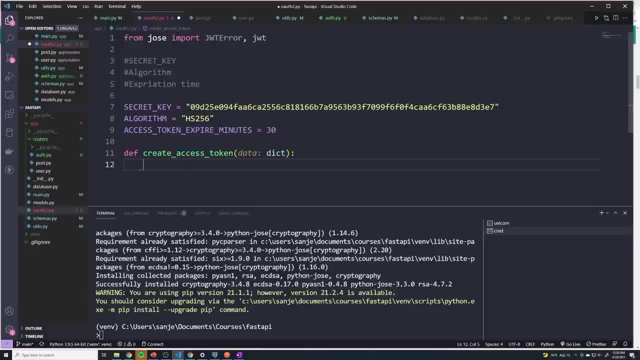 we're going to manipulate a few things And I don't want to accidentally change the original data. So we're going to say data dot copy. So this is going to make a copy. I'm going to store it in. a new variable is going to be to underscore code. So this is all the data that we're going to encode. 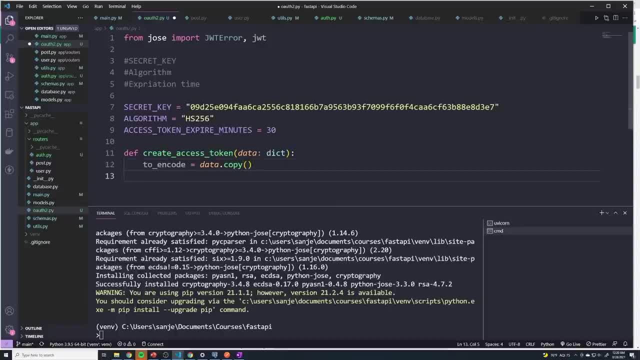 into our JWT token, And then now we're going to create the expiration field. So, to actually do that, there's a couple of things. First, we're going to create the expiration field, So to all, right, now we have it set to 30 minutes, And so what we need to do is to provide the time. 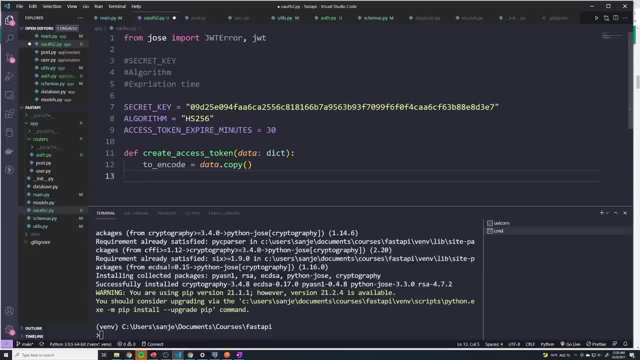 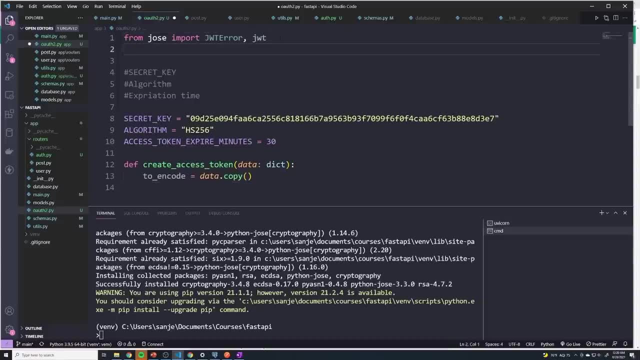 of 30 minutes from now, right, so we have to provide the time that it's going to expire in, So we have to grab the current time and then add 30 minutes, And so anytime you're working with dates and times, we have to import the date time library. 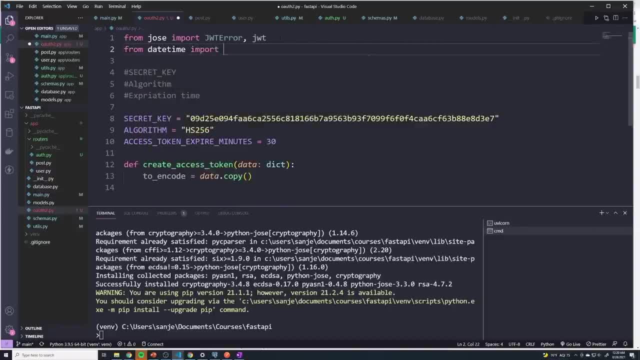 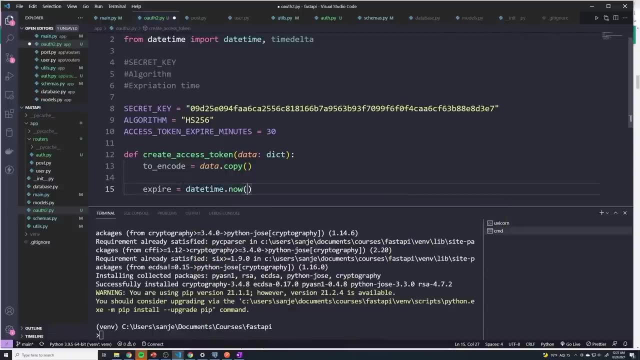 We'll say date time, import, date time and time delta, And I'm going to say expire equals date time dot now. So this is going to grab the current time And I'm going to pass in time delta of, and then, since this is in minutes, I would say minutes equals. 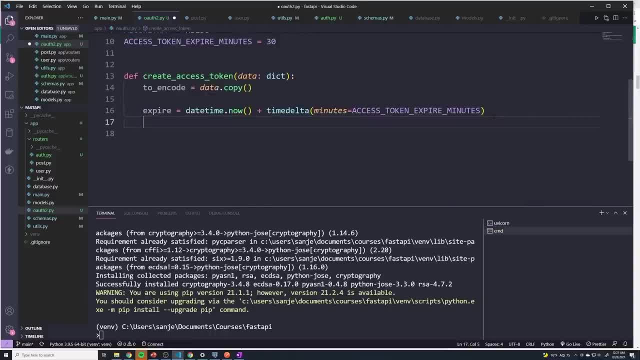 access token expire minutes. And then what we want to do is is we want to grab the to encode, which is a copy of a dictionary. So this is also a dictionary And I want to update it. And here we're going to pass in expiration and then we're going to 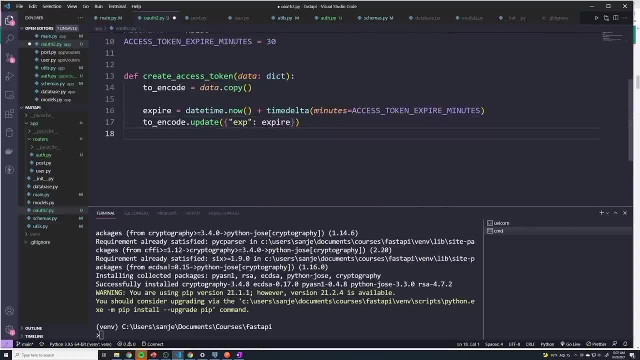 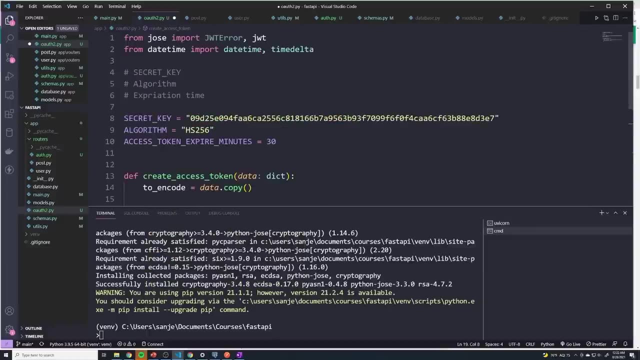 provide the expire time. So we're just adding that extra property into the, into all that data that we want to encode into our JWT, And so now our JWT will tell us when it's going to expire, And what we're going to do is we're going to call JWT coming from the. 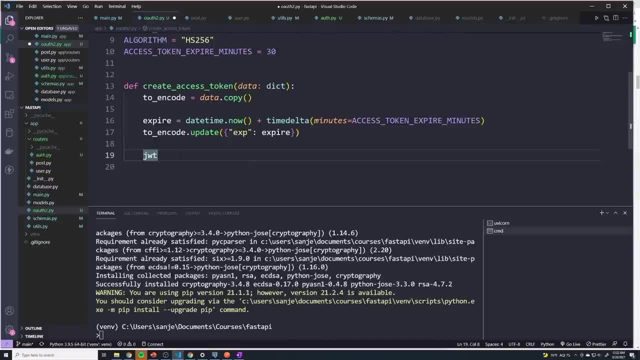 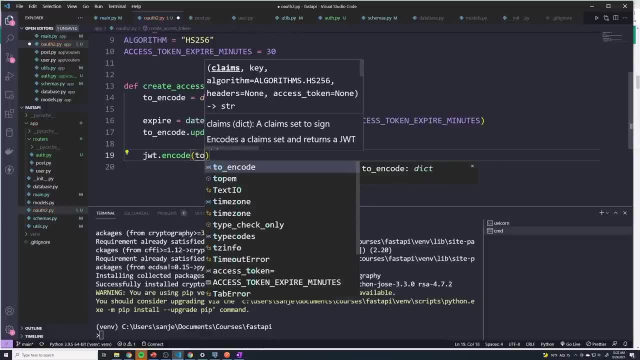 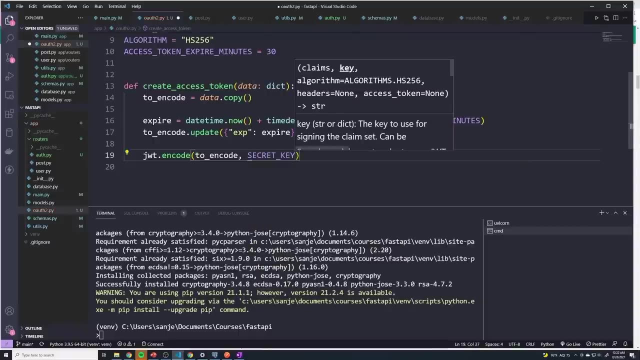 is it Jose? I guess it's the Jose library. So JWT dot encode that. this method is actually going to create the JWT token And we'll say: the first property is everything that we want to put into the payload. The second one is going to be the secret key, the signature, And then we have to. 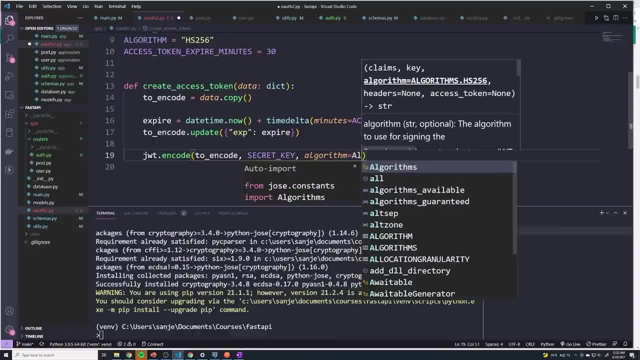 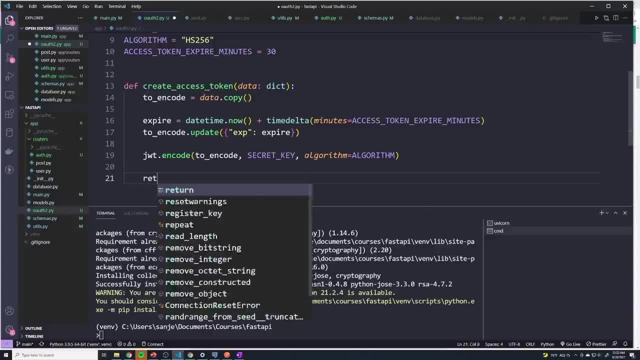 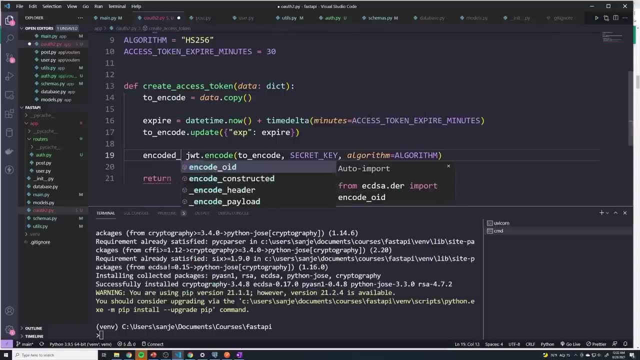 specify the algorithm. the algorithm equals algorithm. I'll go to right there, And at this point we're just going to return. we have to save this in a variable, And here we just doing coded JWT and then now we can go back to our specific path operation. 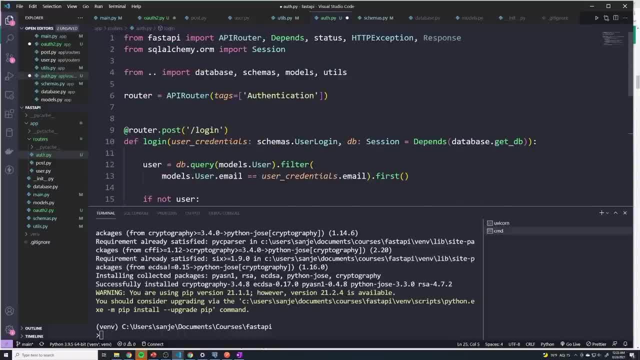 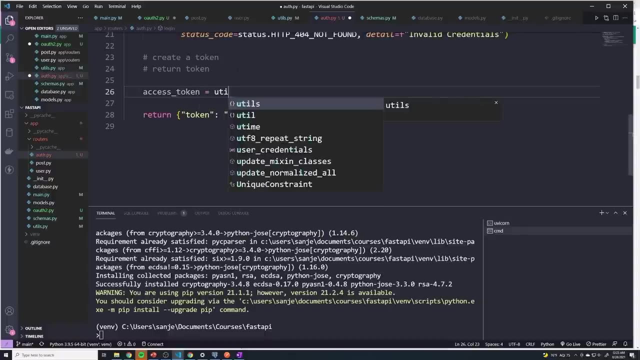 And since we're already importing, actually we have to also import a lot too. And then here we're going to create an access token And we're going to call the sorry, not utils a lot to dot create access token. I'm going to say the data equals. and then we're going 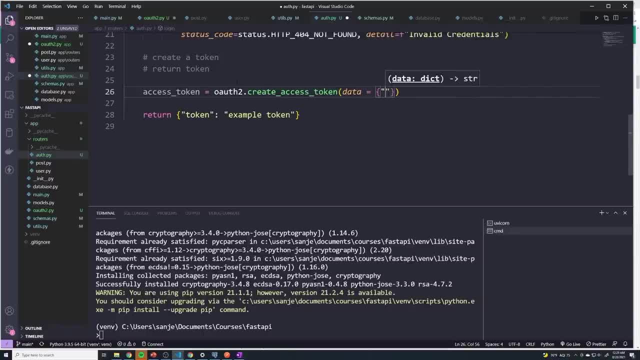 to pass in a dictionary. So here the user ID. Remember, this is the data that we want to put in the payload. So I have decided that I'm going to put in the user ID and pretty much nothing else. I don't really care about anything else. we could give it a role. we. 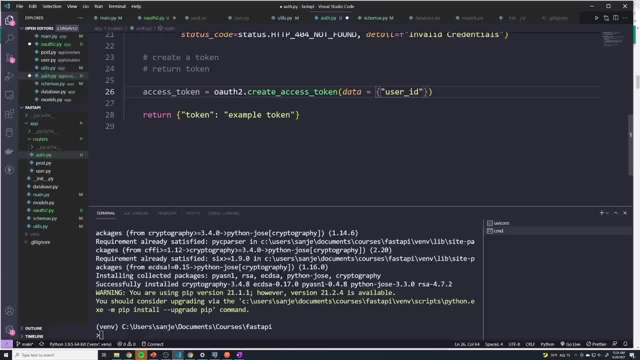 can do something else, But for me, I just want to encode the user ID, So that's what I'm passing in here. However, if you wanted to provide some extra information about the user, if you wanted to provide, you know their scope of. 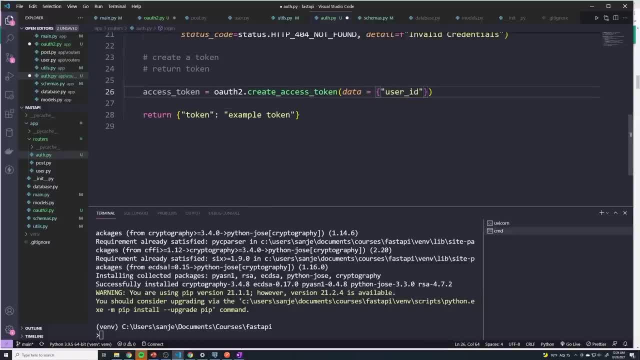 different endpoints they can access. you can put all of that information in here. And so I'm gonna say the user ID is going to be set to user dot ID. And so now what we can do is we're going to return a few things. I'm going to say we're going to return the 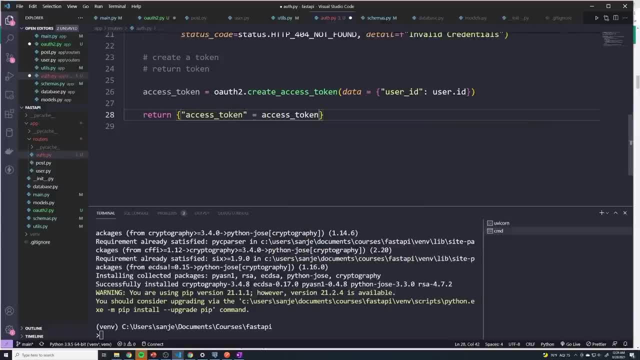 access token, which equals access token, And then we're going to tell the user what kind of token this is. So this is token underscore type And this is what's referred to as a bearer token, And I'll explain how to actually configure that on the front end. But literally, 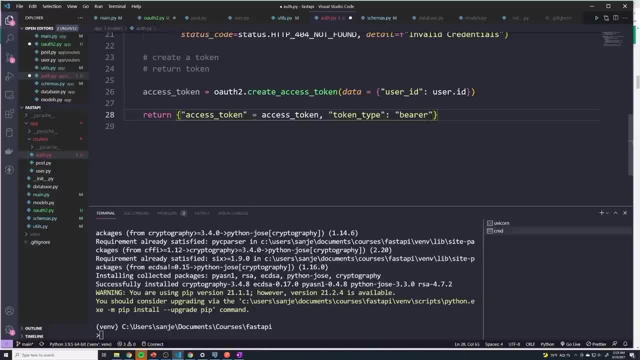 in the authorization header we just write the word bearer and then we provide the token. So nothing special there. All right, let's try that out. And it looks like I got an error And I don't know why. I put an equal. 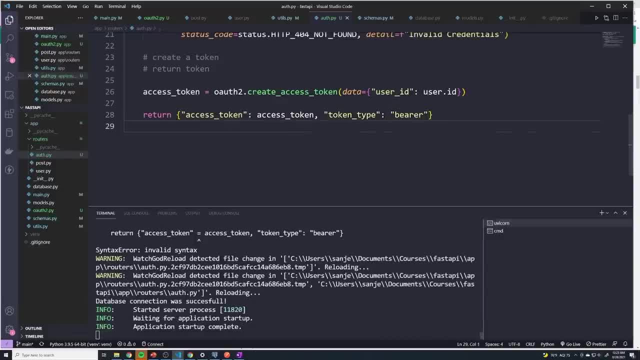 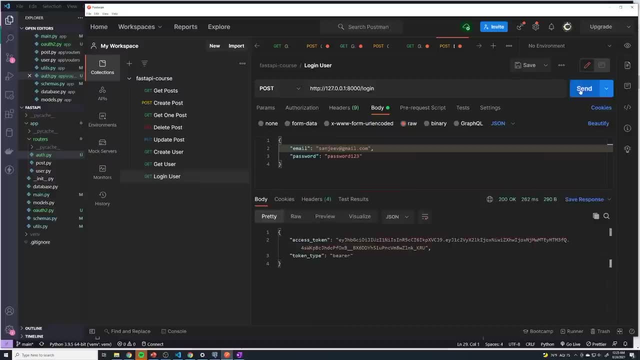 sign there And let's try this out. So we've got. we've got the login endpoint. let's put in the correct email this time And let's see what happens. Look at that. we got an access token And this kind of looks like a JWT token. right, It just looks like a bunch. 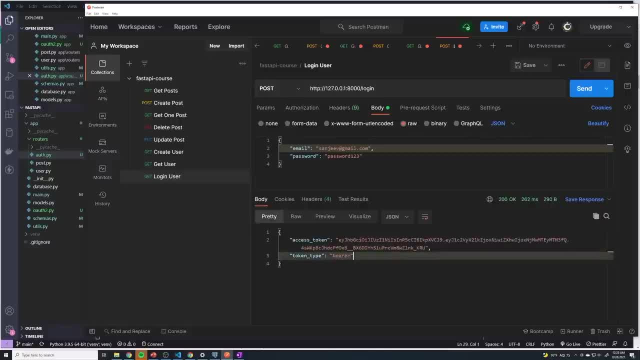 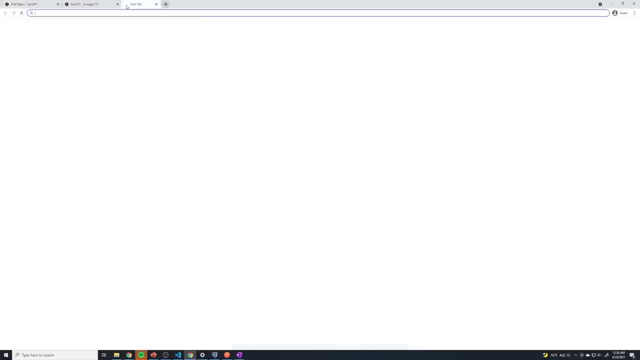 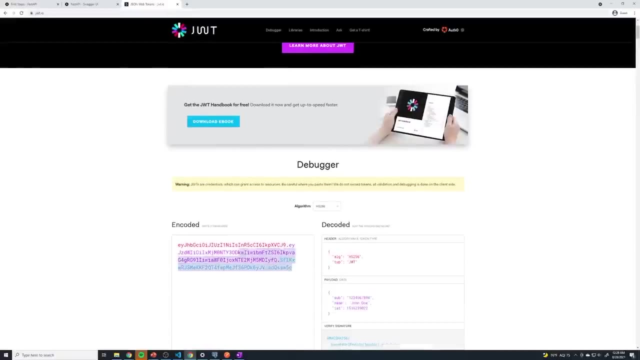 of random text And then it tells us it's a bearer token. So let's actually copy this. And what I want you guys to do is go to your web browser And I want you to search for JWT And then go to the first one, go to JWTio, And then here, what we can do is we can paste. 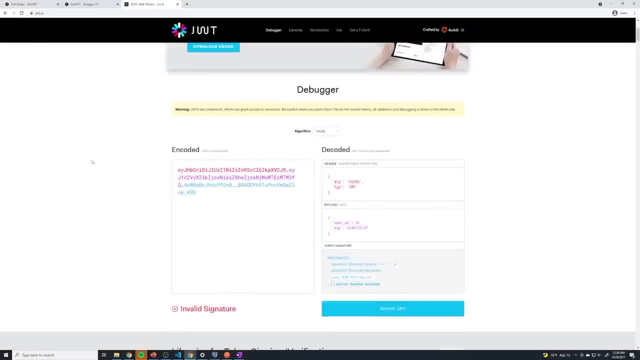 in our JWT token, And what's really cool is it's going to decode the token for us, And so you can see this is the algorithm we use. it is a JWT token, But take a look at the user ID. Right, This is the actual user ID that we passed into the token. So all of the 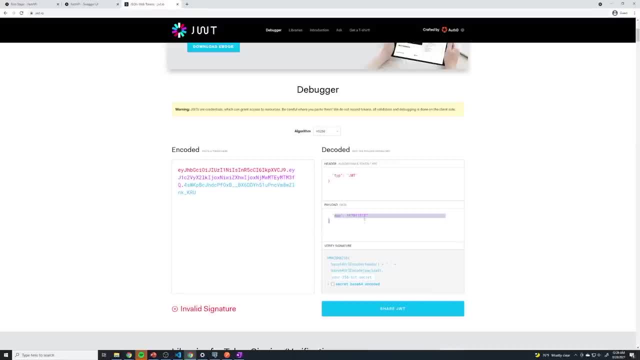 data that we encrypted into the token. we're going to be able to decode that into the token, And then we're going to go to the first one, we're going to go to the second one, we're going to go to the token. are all sitting right here, So we also got the expiration. 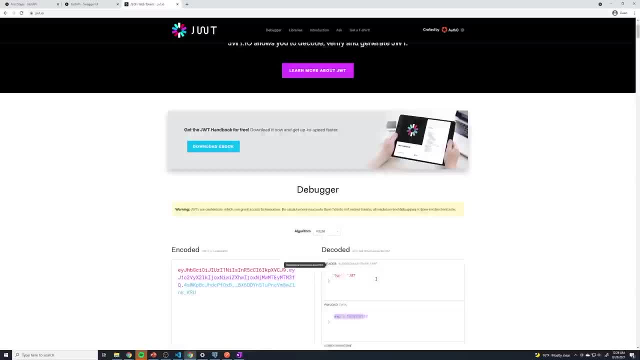 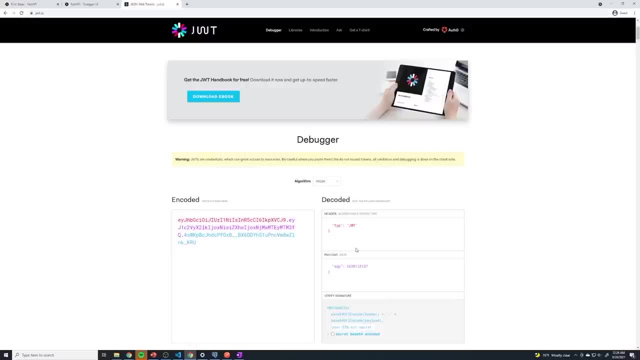 time, And then the signature somewhere in here as well. But isn't that pretty cool, right? It was able to decode it And it's important to understand that. you know. none of this is encrypted. anybody can see this information- But by being able to sign it, 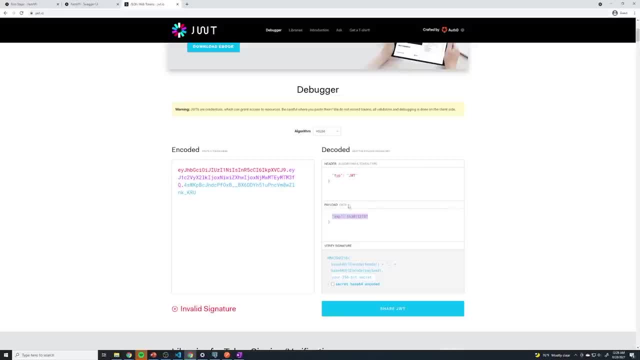 we know that no one can kind of mess with it And we can also specify an expiration time, So we know that how long this token is valid. So when the the our API gets it, it's going to just verify that nobody touched the token. it's going to verify that hey. 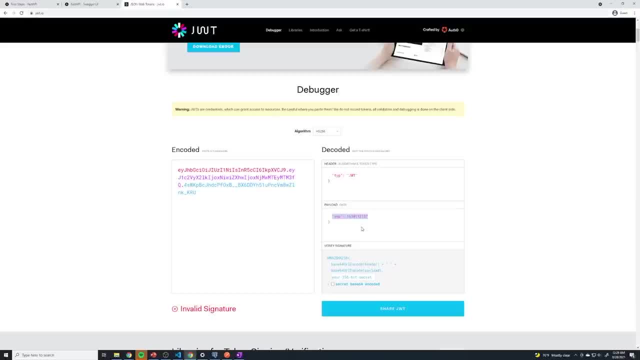 hey, the expiration time isn't before the current time, which would mean that it's already expired. At that point it already knows the token's valid, and then we can assume that everything is good to go. We're going to make one small change. 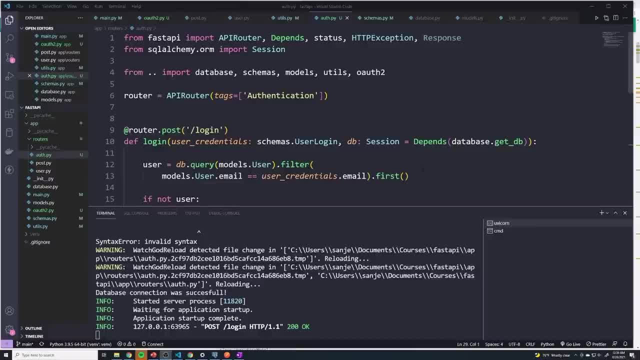 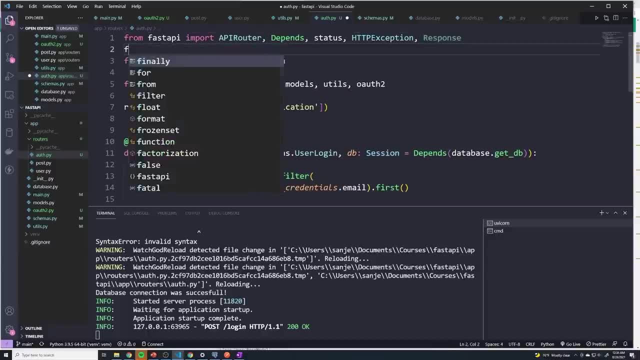 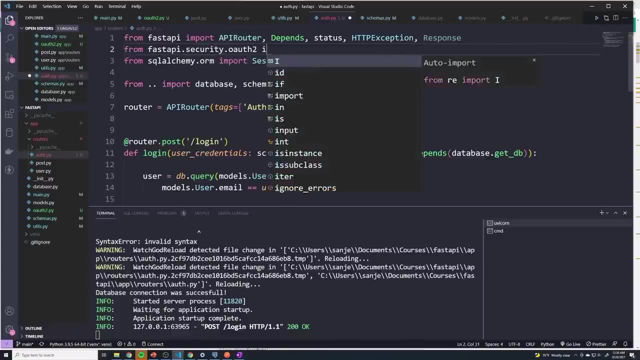 when it comes to retrieving the user's credentials in our login route, Instead of passing it in the body, we're going to use a built-in utility in the FastAPI library. So if we do from FastAPIsecurityoauth2, we're going to import something called. 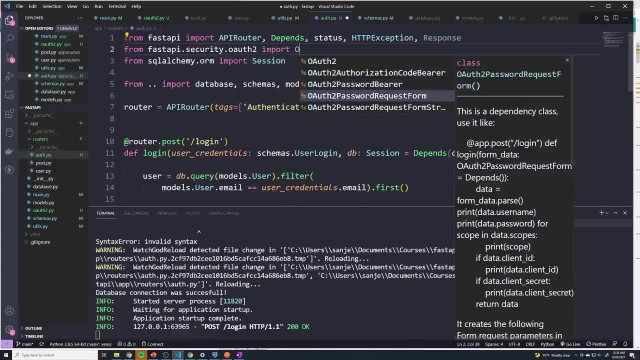 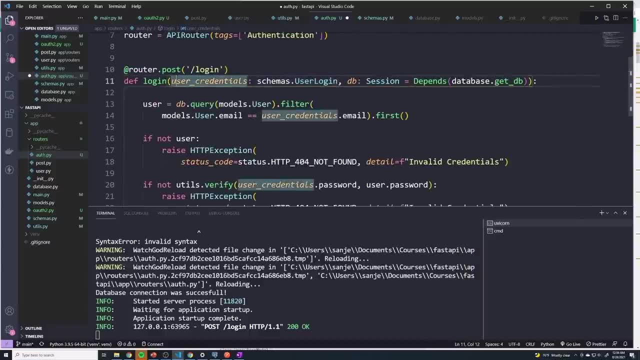 oauth2-password-request-form, And so what we can actually do is, instead of just doing the usual here with the user credentials, we're actually going to delete that and I'm going to provide a dependency. Well, actually I need the user's credentials. 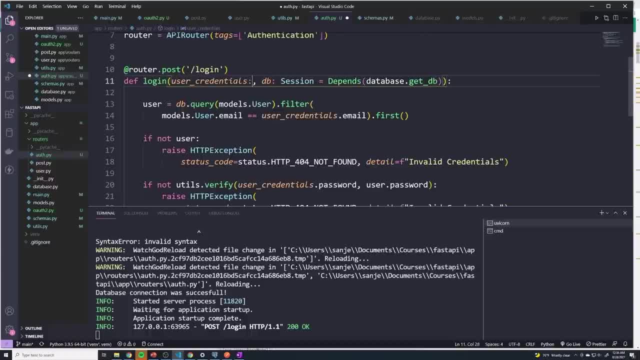 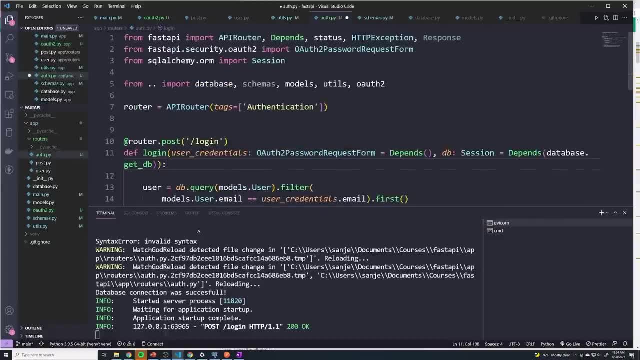 because we have to store it someplace. But here we say this: equals oauth2-password-request-form, equals depend. So we're setting up a dependency, kind of like we do with the database, and so this is going to require us to retrieve the credentials. 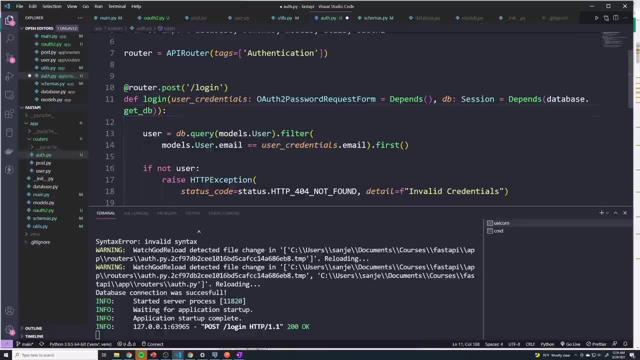 and then FastAPI is automatically going to store it inside this variable called userCredentials. However, we have to make one small change, So the username. when you retrieve the user's attempted credentials from here, what it's going to do is it's going to store it. 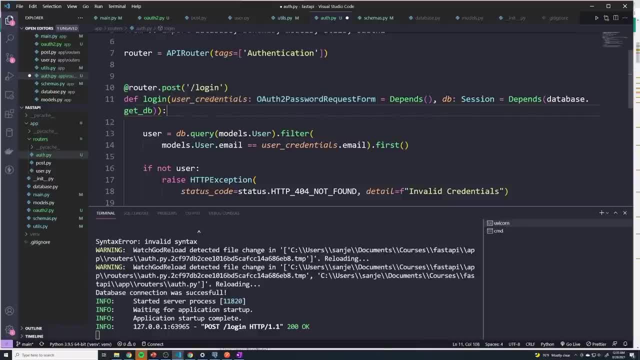 in a field not called email, but it's going to store it in a field called username. So when we compare the modelsuser at email when we're querying the database, we can't compare it to user underscore credentials Email, because there's no field called that email, right? 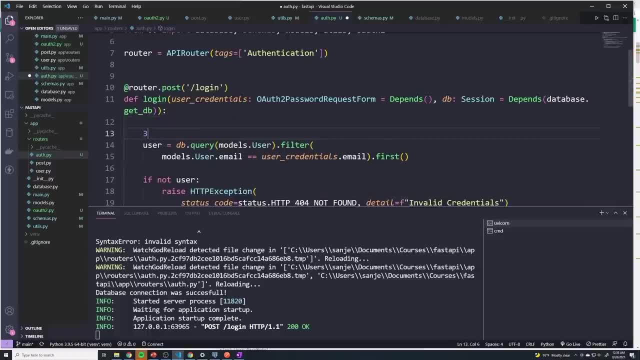 It's going to only return two things. It's going to return Oops, it's going to return something. It's going to return our username, which equals whatever, and then it's going to return our password, Which equals whatever, And so we don't have access to email. 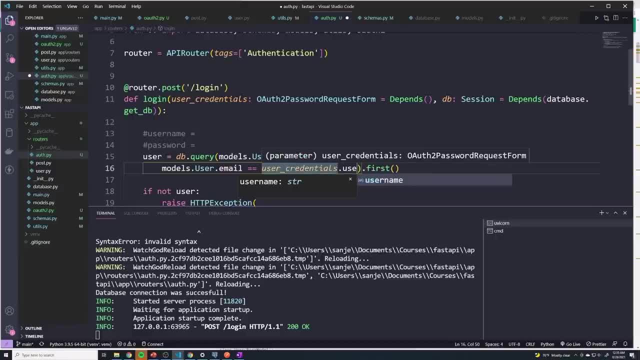 We have to use user dot- sorry, user underscore credentials dot username. because, well, this is actually a bad example, because you have to think of it as like a dictionary. right, It's going to be like a dictionary. It's coming in like this: 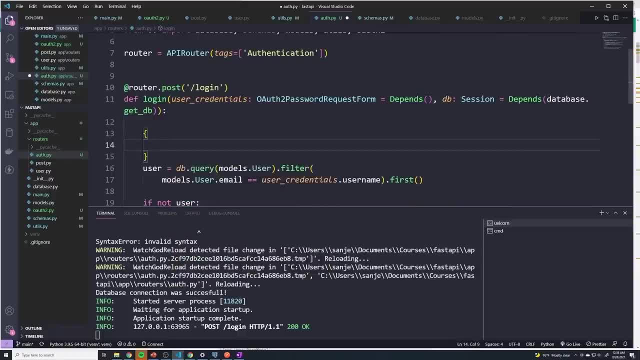 and then there's going to be a user field. You're going to have username- Oh, why is that capitalized? Username, which equals blah. You're going to have username which equals, you know, blah. and then you're going to have password. 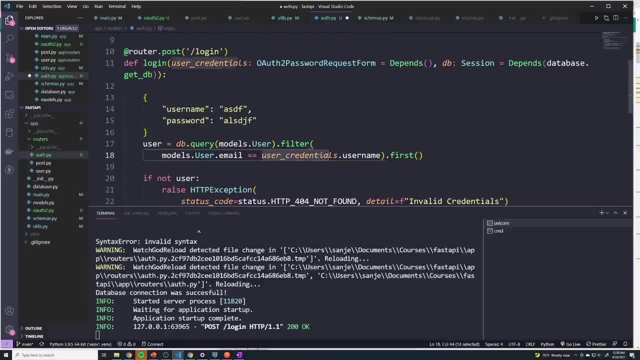 which equals blah, right, And so we'll just tag user credentials, dot, and then we'll grab the username, which in our case will happen to be the email. The OAuth 2 password request doesn't really care what the username is. 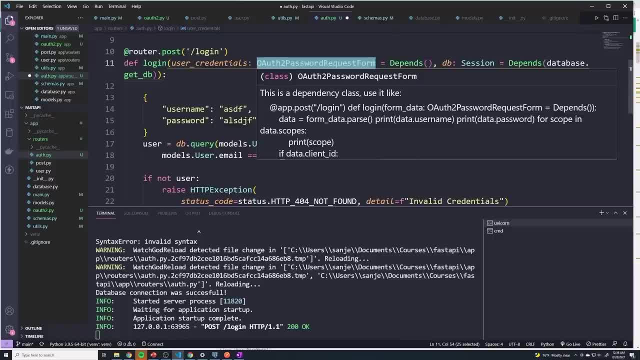 It could be a username, It can be a email, It can be an ID, It doesn't really matter, It doesn't really care, It's just whatever the user actually sends. It's just going to store it in a field called username. 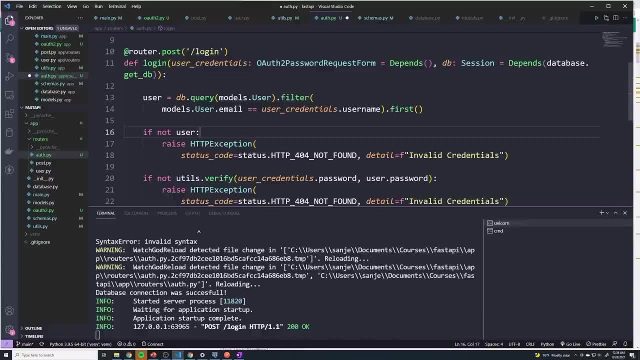 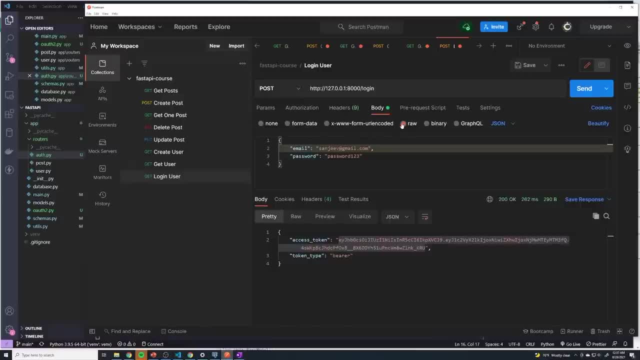 So those are all of the changes that we have to make from our backend side. Now, when it comes to testing things, we no longer send the credentials in the body like we normally do. Like, if I try to send this now, we're going to get an error, right. 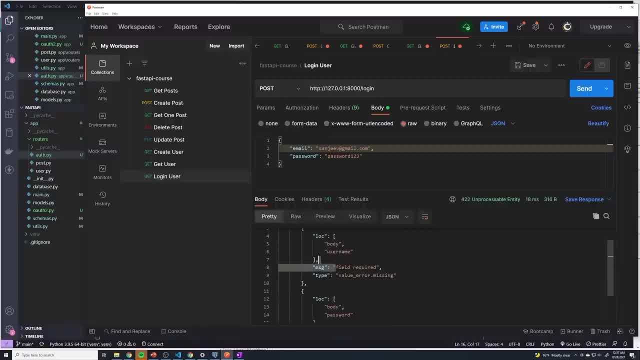 Because it says username Is field required, value error missing. So what we? and the password is also missing. So what it's doing is it no longer expects it here. Instead it expects it inside form data. So here I'm going to say username. 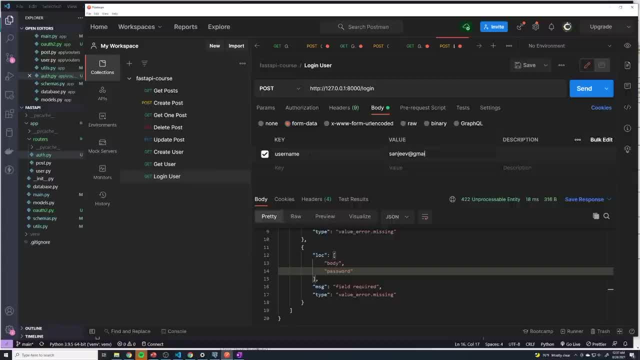 and this is going to be my email in this case, And then my password here, And so let's try this now And now it successfully works. So those were the couple of changes that we have to make, But you'll see that it makes life a little bit easier. 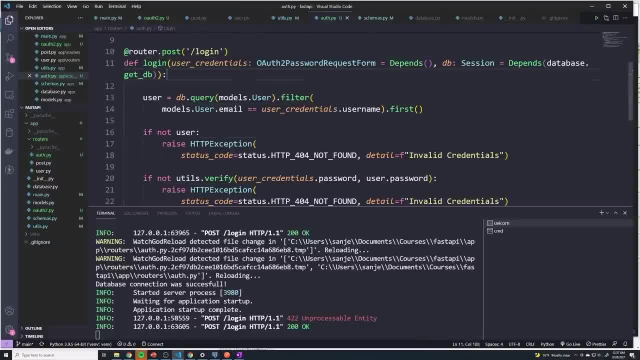 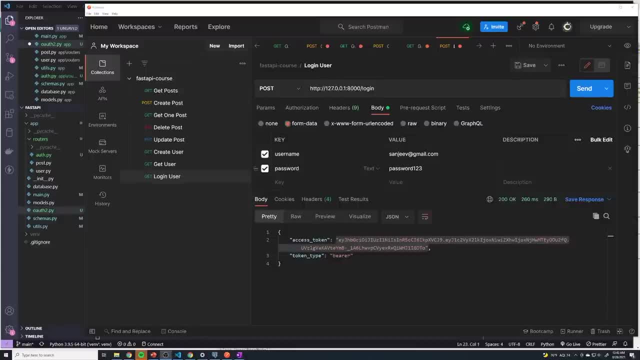 by setting up that dependency and using the built-in functionality of FastAPI. In the last lesson, we learned how to log in a user by sending a request to the login endpoint and providing the username and password, And our API will then return an access token. 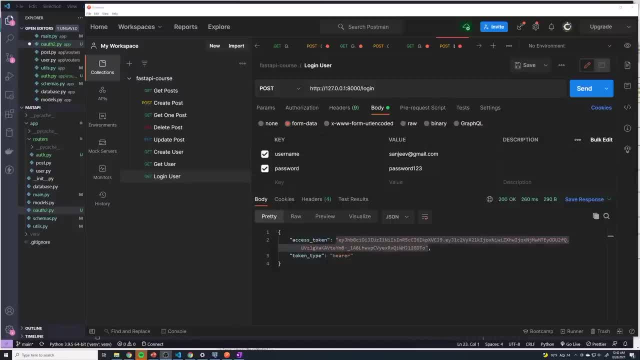 which the user can then use to retrieve data from our API. So anytime he needs to access a endpoint or a path operation that requires a user to be logged in, he'll just send this JWT token in the payload And then our API has to actually validate the token. 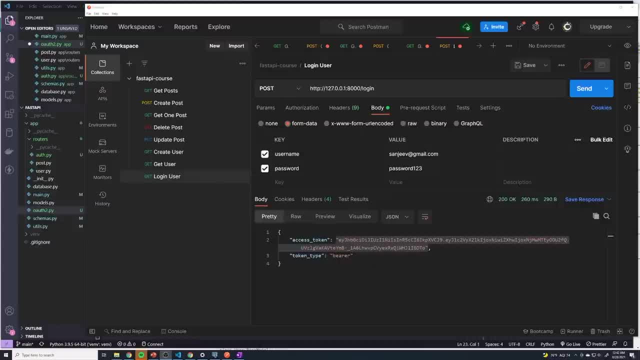 So in this video, we're going to handle the logic for verifying that the token is still valid and that they didn't tamper with it, as well as verifying that the token hasn't expired. Now, before we do anything, what we're actually going to do is 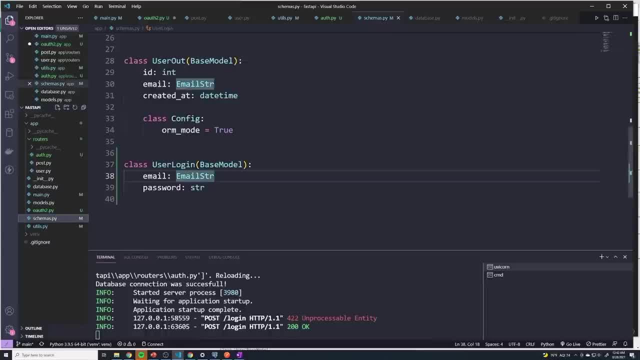 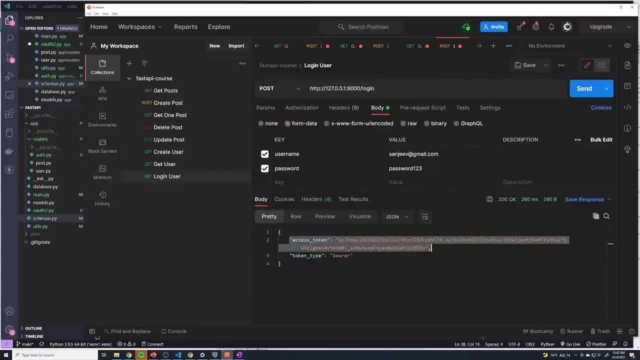 we're going to define a schema for the token because we know that the user has to provide the access token. So, just like any other piece of data, if we expect them to send something, it's best to set up a schema. So we're just going to set up a schema for access token and token type. 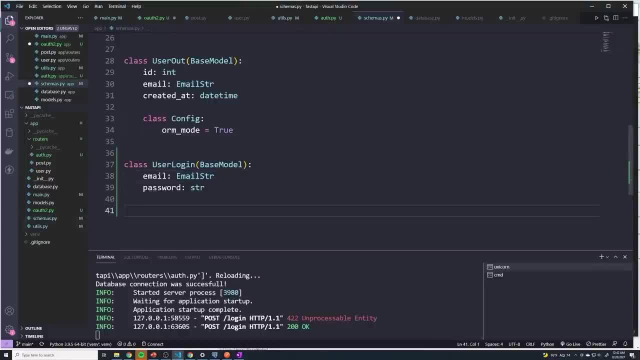 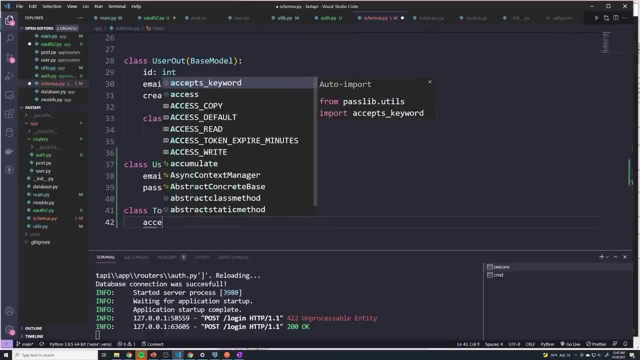 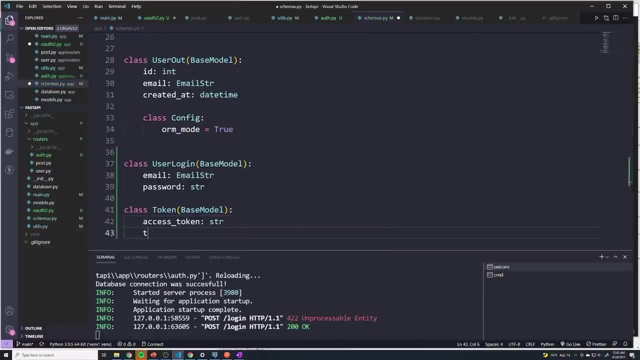 and just make sure that they match accordingly. And so here we're going to do class token And we'll say: the access token is going to be up type string And the token underscore type is going to be up type string as well. And then we can also set up a. 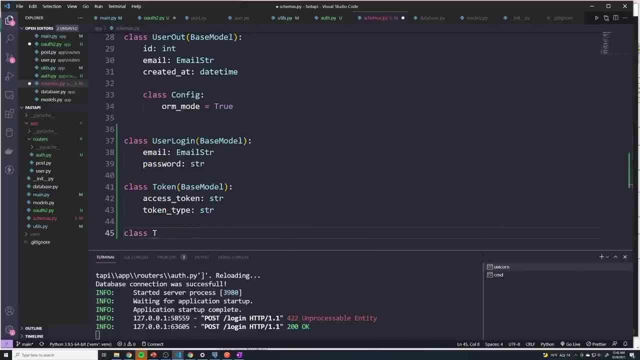 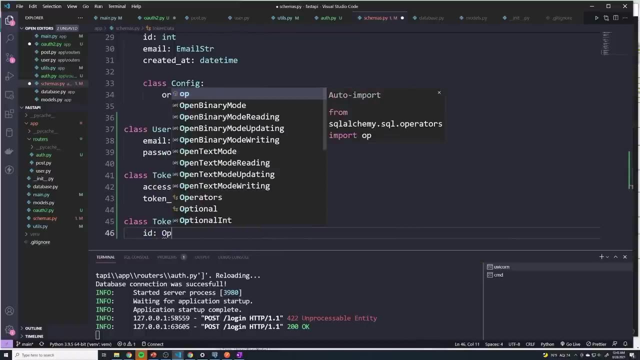 a schema for the token data, So that the data that we embedded into our access token, so we can say token data base model, And then here we did embed the ID, But I'm going to say this is optional for now. 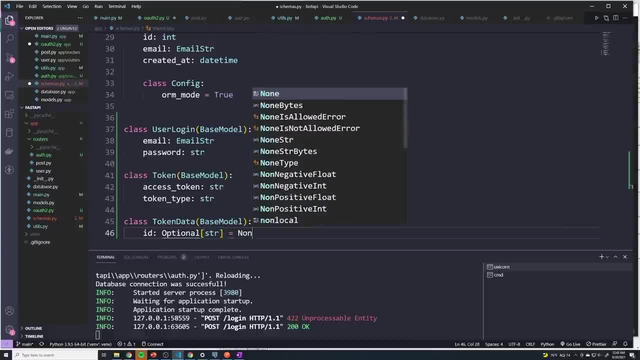 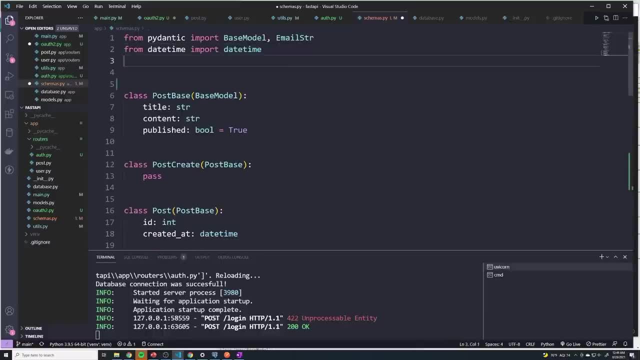 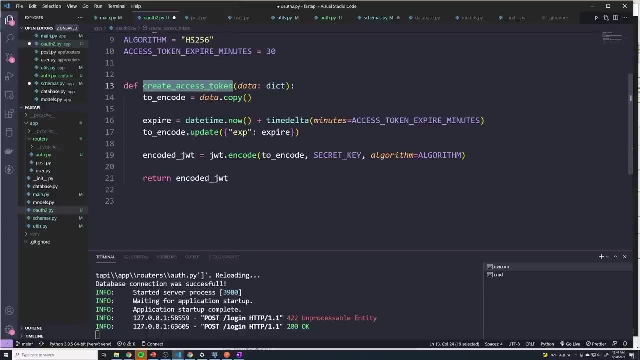 And it's gonna be a type of string, if it is set, So it can be optional, and we got to import optional as well, And so that's going to come from the typing library. And then in our OAuth two file we created an access token function. 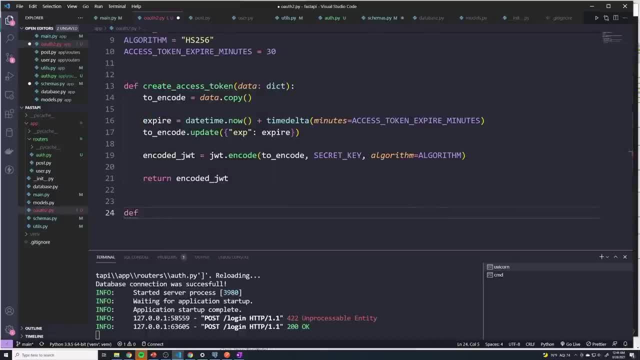 And then we have to create a function to verify the access token. So let's create the function, and it's going to just be called verify access token, And what we're going to do is we're going to pass in a token which is going to be a string. 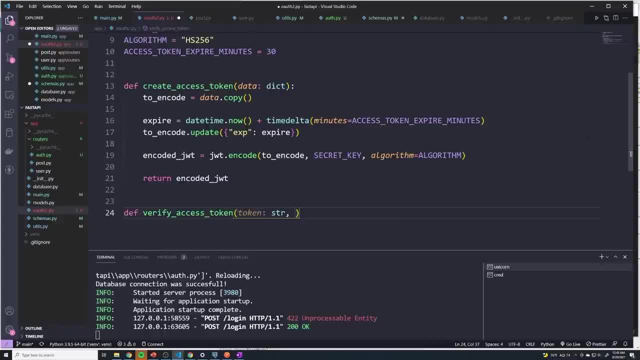 And we're also going to pass in the specific credential exception. So we're going to pass in a string And we're going to pass in what our exception should be if the credentials don't match or if there's some issue with the token. 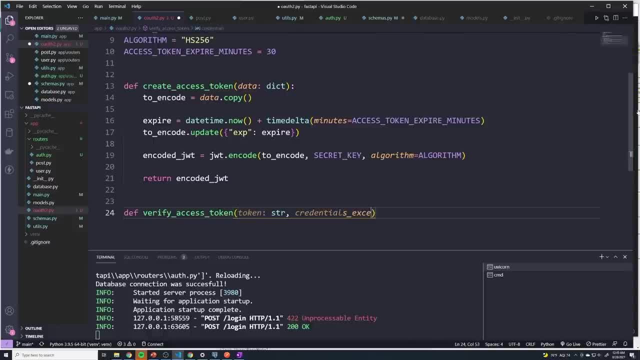 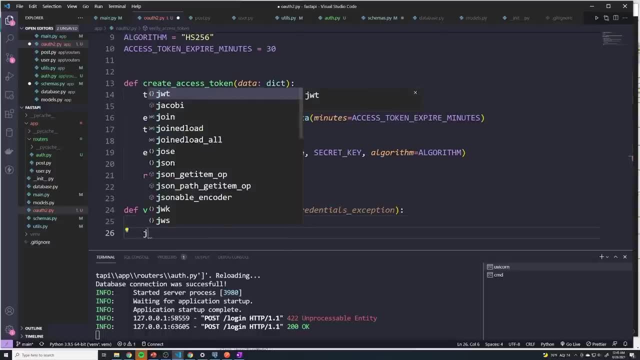 So we'll just store this in a variable called credentials underscore exception, And I'll explain this a little bit later. And so here I'm going to say JWT- right, so we're going to access the JWT library. I'm going to say JWT dot, and it's going to have a function. 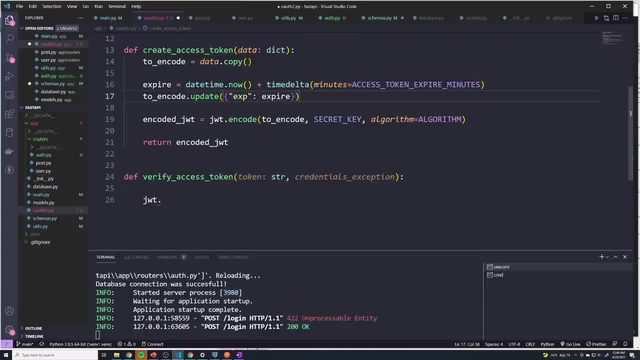 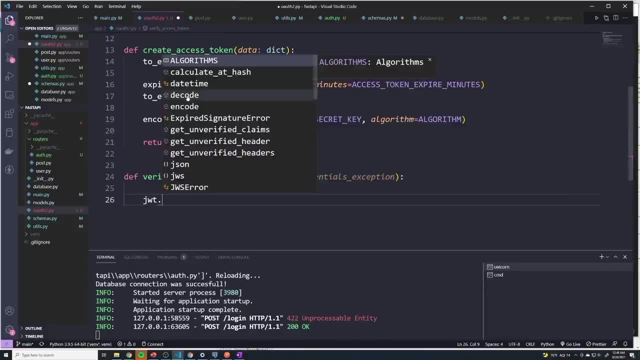 And if you take a look at our options, I'm sure you have an idea, because, creating a token, we did encode dot, encode dot. I'm guessing you can figure out what is the specific method for decoding. it's going to be decode, obviously. 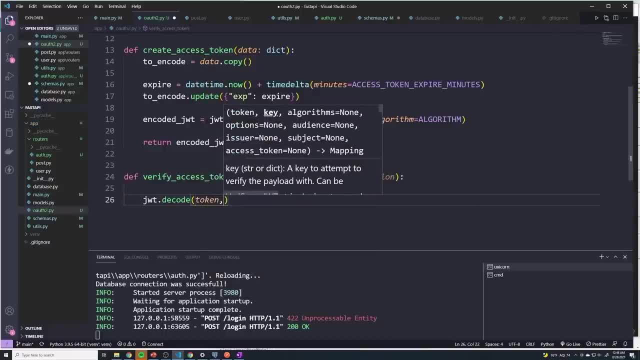 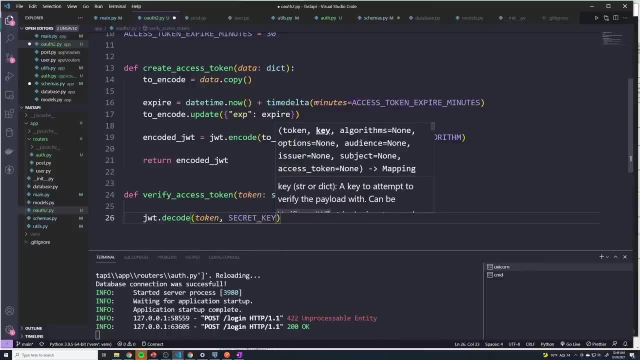 And here we're going to pass in a couple things. First of all the token. then we have to pass in the secret key so that we can decode it, And then we have to pass in the algorithm that's used, So we can just pass an algorithm. 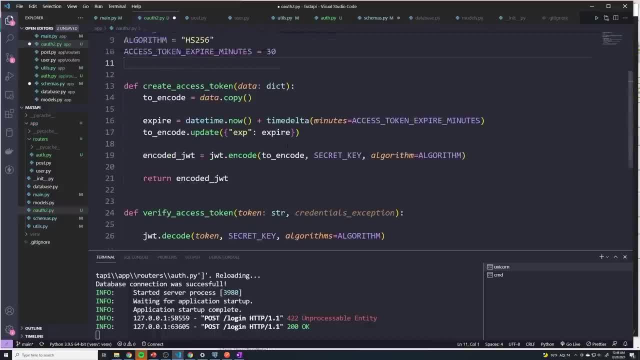 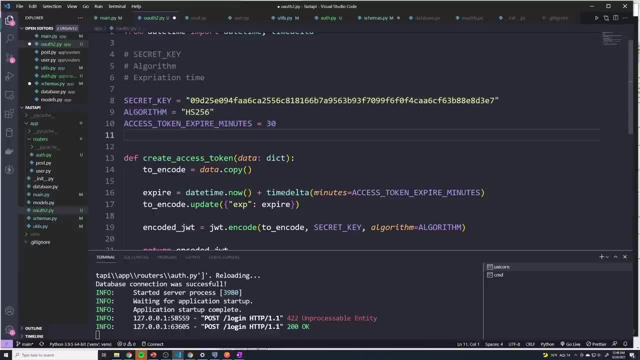 Once again, these. both of these are coming from these variables right here, Not all of them. It's obviously not a good idea to store the secret key within your actual code But, like I said, we're going to have a later section where we'll turn these into environment. 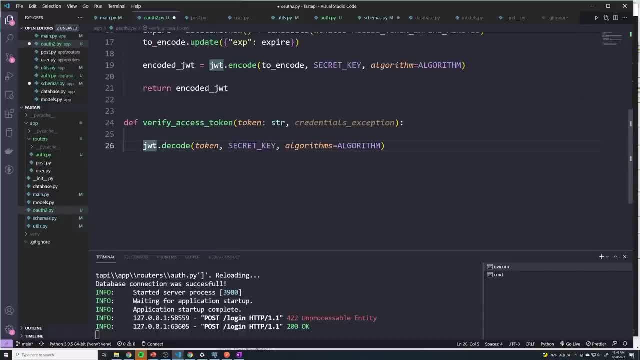 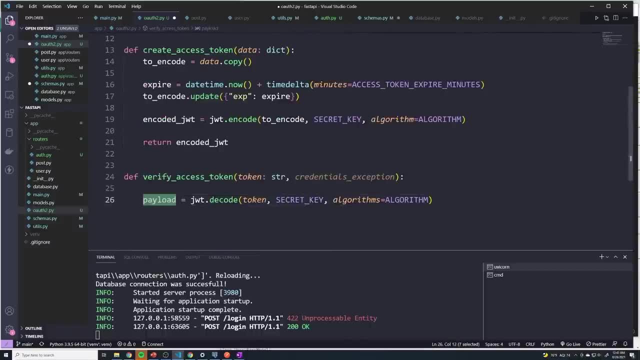 variables, so that it's not hard coded into our code, And we're going to store this in payload, in a variable called payload, And so this will just store all of our payload data. And to extract the data what we can do is we can say payload dot- get and then we have to get the specific. 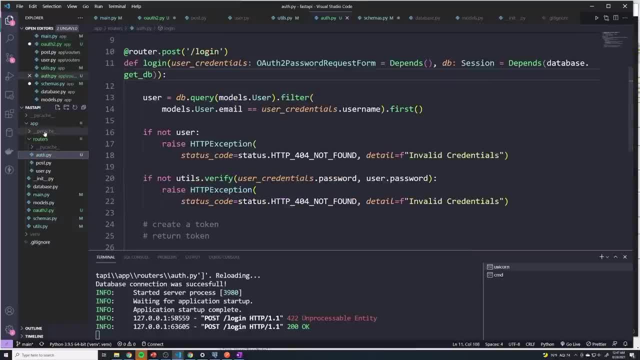 field that we put in. So if I go back, I'm going to go back to my code and I'm going to go back to my auth dot py file in my routers. And you take a look at my data, you can see that we have a field. 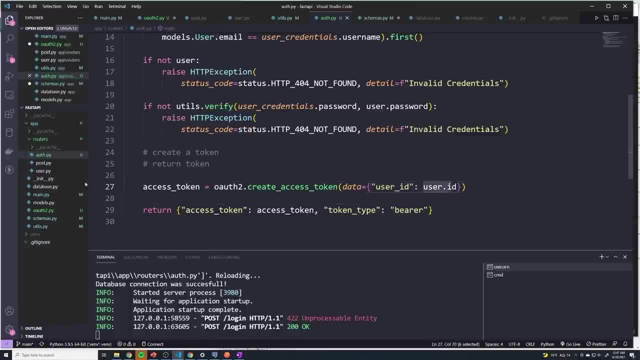 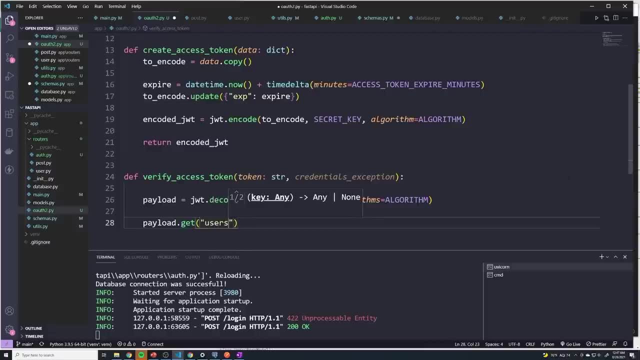 called user underscore ID And that's going to get the ID of the user. So here we just say get, And then we just pass in that same exact name, users underscore ID, And we'll say that this is going to be stored in a variable called ID. 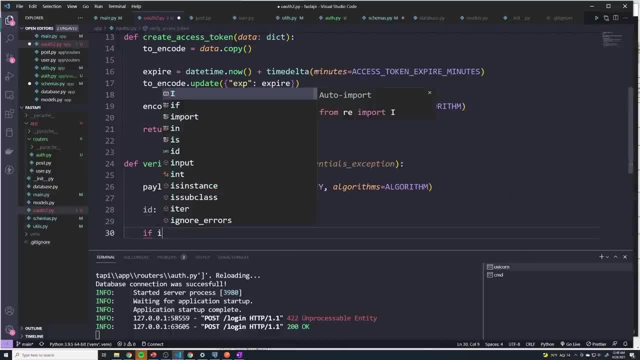 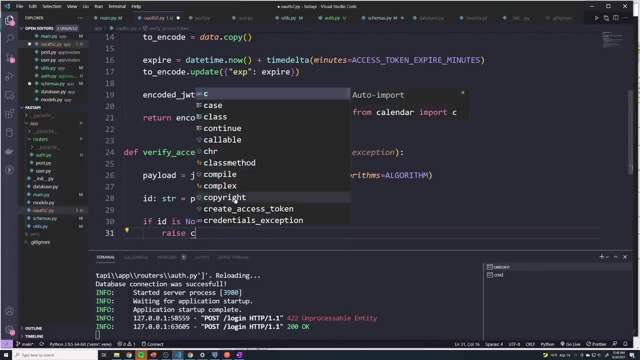 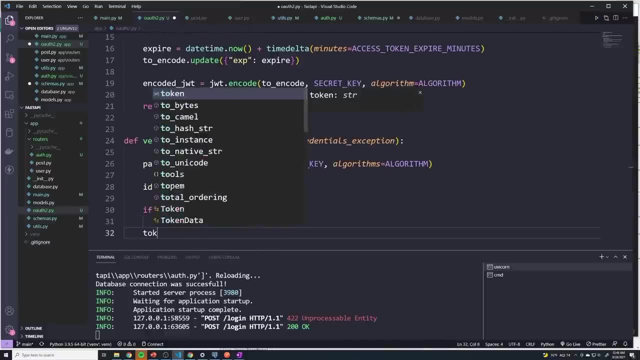 And this should be of type string. And if there's no ID, then we're going to raise a credentials exception, Right? so whatever exception we provided into this function, it's going to raise that. And then we're going to say: token underscore data equals schemas dot. 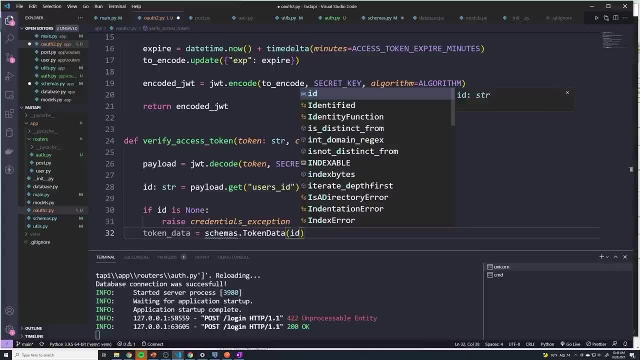 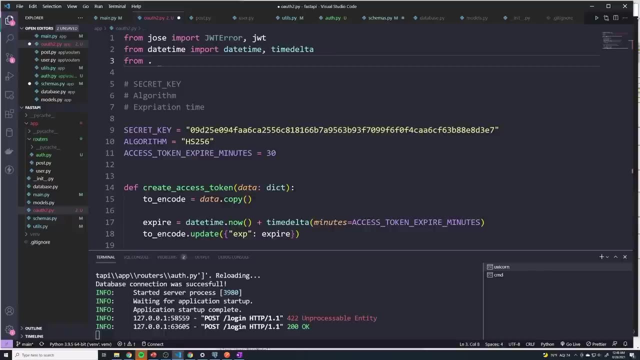 token data with the ID equals the ID that we extracted out of here And I see that we didn't import schema, So I'll import that real quick. We'll say from dot import schemas, And so all this is going to do is it's just going to validate. 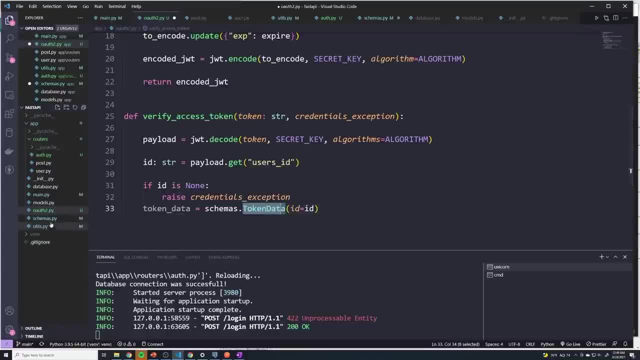 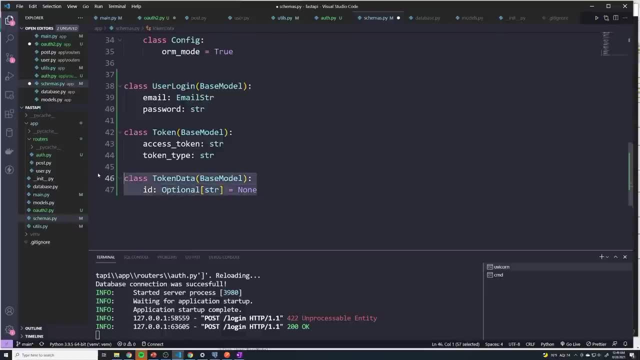 you know that it matches our specific token schema. Now, if you look at our schema, right, it's literally one thing, So it's not super exciting, And I made it optional. So we shouldn't actually make it optional, But we'll come back to fixing this in a bit. 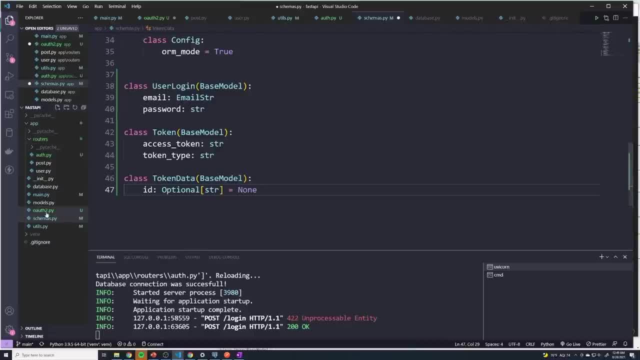 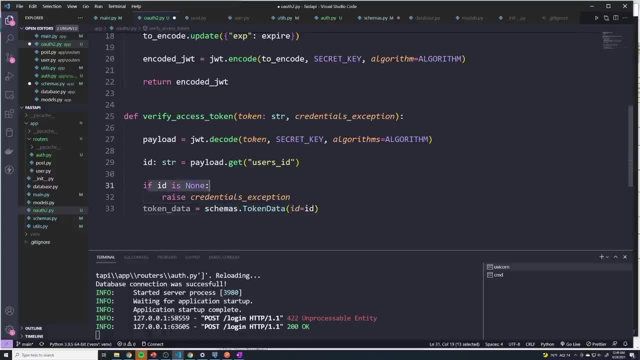 But this is just going to ensure that all the data we pass in the token is actually there, And so that's why I'm using a schema for that. However, for one actual variable, you don't actually need to do that, especially since we're checking to. 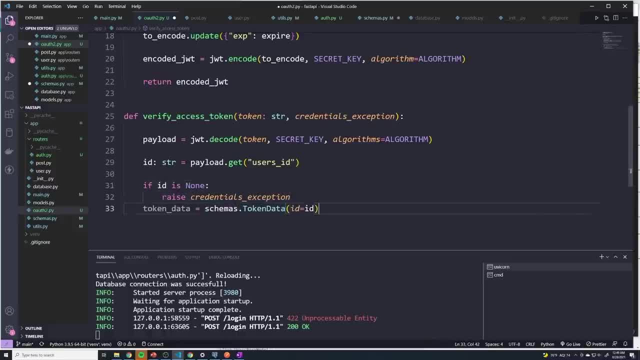 see if it exists right here, But it's good to always make sure. so in the future, if we do add extra fields, we can also validate the schema here. Now we're almost done with this function. However, there's one little issue, because we can run into an error in any one of these lines And 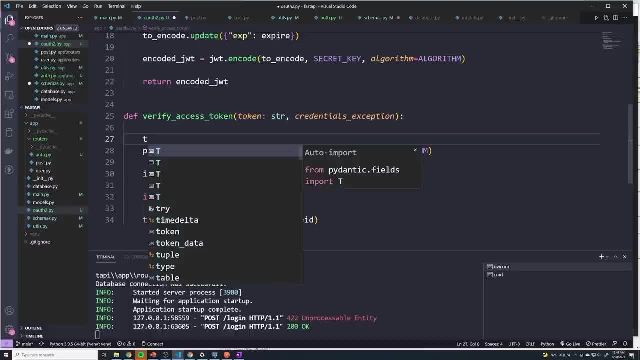 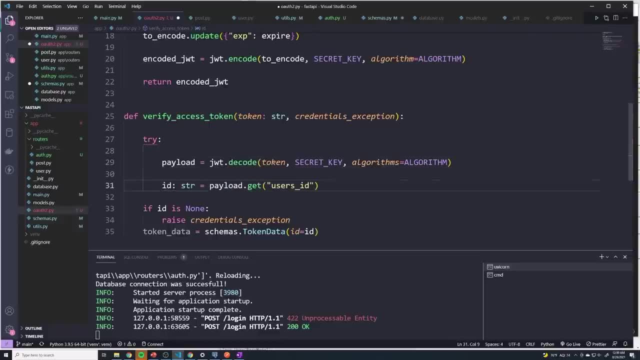 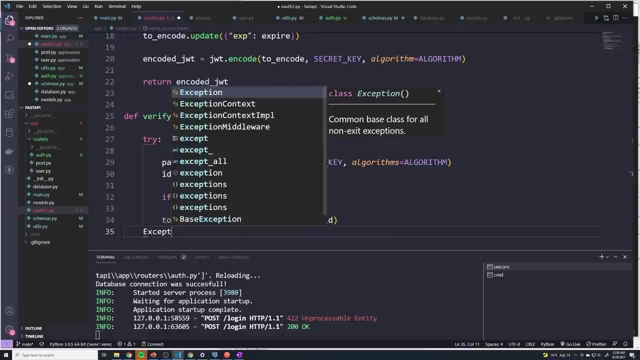 so anytime you're working with code that can error out, you want to do a try except block. So we'll do try And then I'm going to indent these And then here we'll say accept And I'm going to pass JWT error. 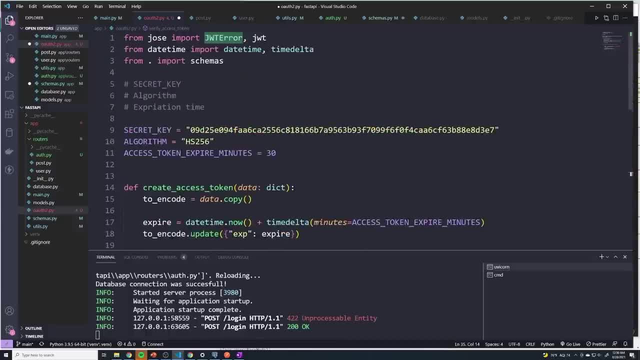 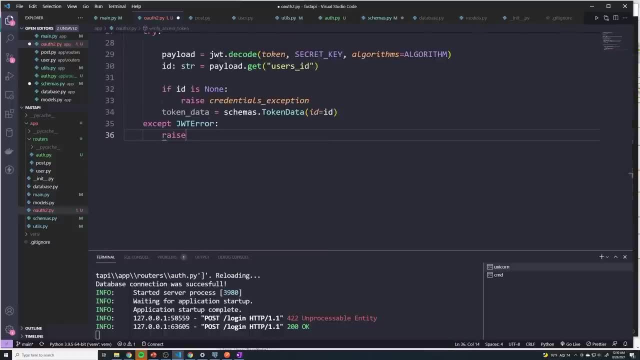 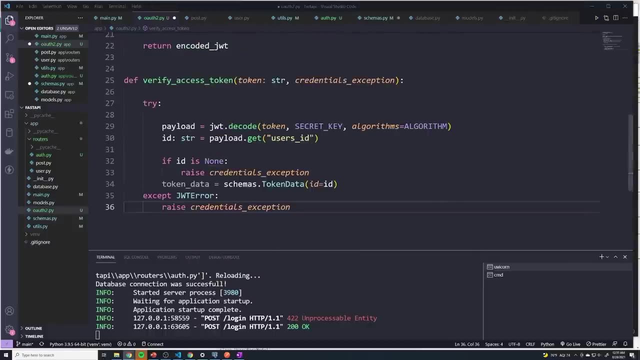 And this should not be capitalized. And remember, this is coming from the Jose library And once again, we're just going to raise a credentials exception If there's any kind of error that we didn't account for I, and the next thing that we have to do is define one last function. 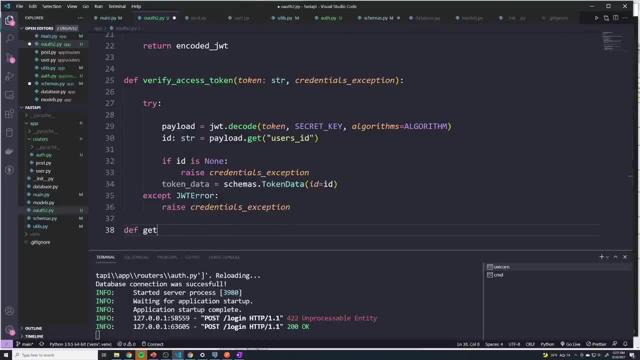 And this is going to be called get current user. So what this is going to do is- and so what this is ultimately going to do- is that we can pass this as a dependency into any one of our path operations, And when we do that, what it's going to do is it's going to 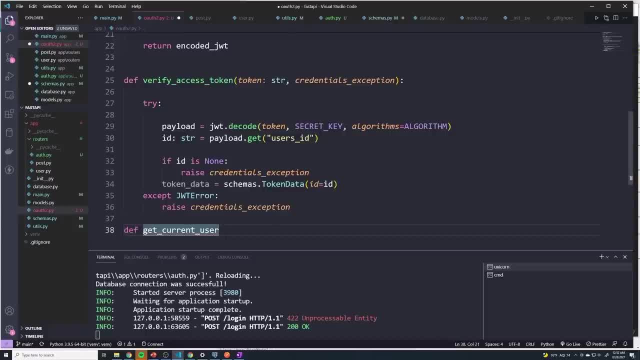 take the token from the request, automatically extract the ID. for us It's going to well. it's going to verify that the token is correct by calling the verify access token And then it's going to extract the ID And then, if we want to, we can have it. 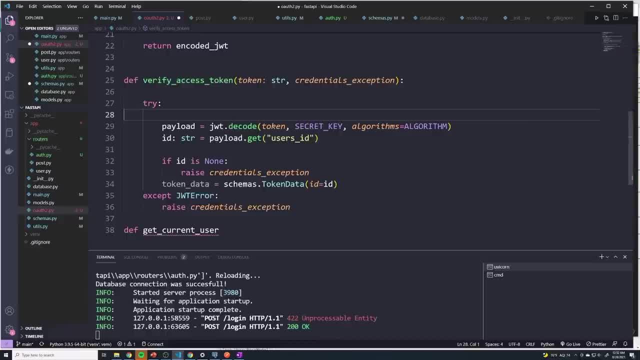 automatically fetch the user from the database and then add it into as a parameter into our path operation function. So here, all we're going to do is we're going to pass the token, And so we're going to actually go ahead, and now we're going to just make sure that there's no error here, THIS TRIPLE ACTIVE 통, And then, if we want to, we can have it automatically fetch the user to boiler paste, so when we're done we can kind of index that And then, if that's the case, let's say let's tack that nodes. 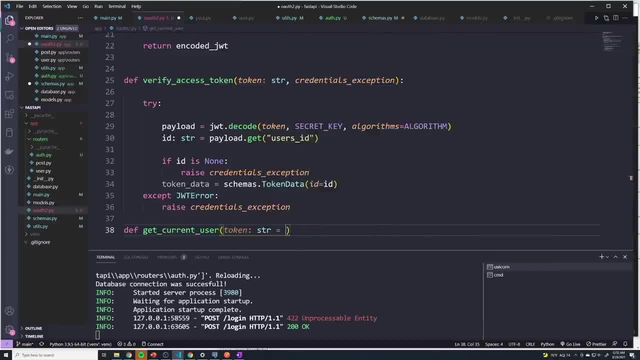 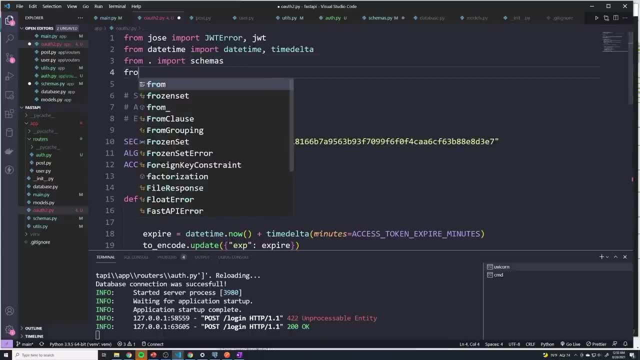 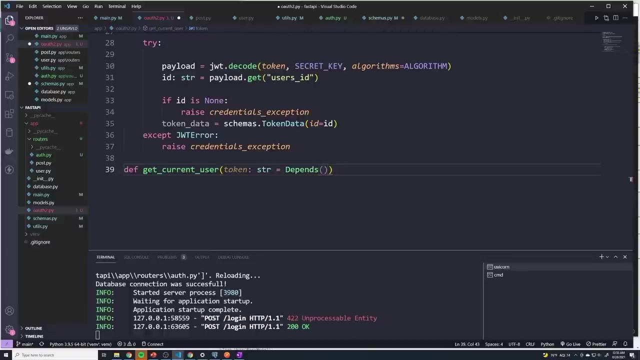 And so this is going to be a type string And then here we just say depends, which has to be imported from the fast API library. So we'll say from fast API import, we're going to import. depends, status and HTTP exception. So here we'll say depends, and then we'll pass in a OAuth two. 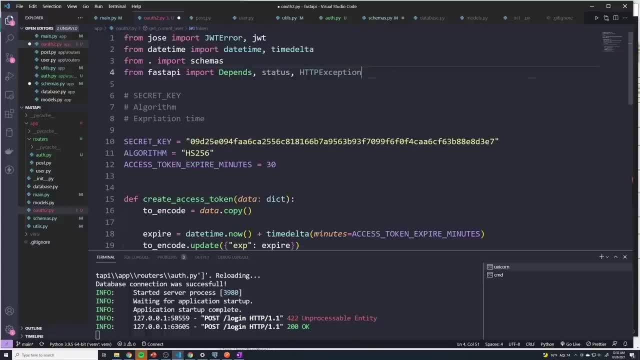 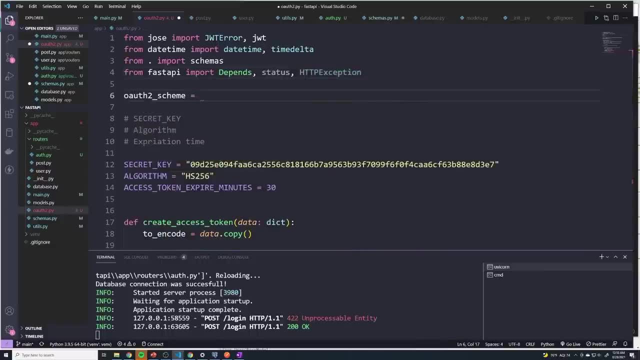 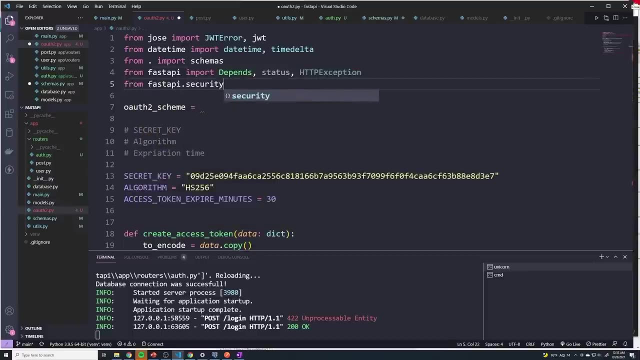 schema or OAuth two scheme. So what we have to do here is- it's gonna be a little confusing- Say a lot to underscore scheme And this is going to be equal to and we have to import one more thing. So we'll say: from fast API, dot security, Import a lot to password bear, And then here 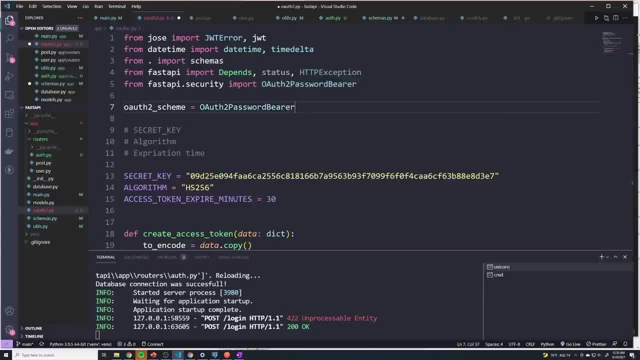 we just reference a lot to password bear, And what we have to do here is we have to import a lot to password bear, And what we have to do here is we have to do is we have to provide one field called token URL, And so this is going to be the the endpoint. 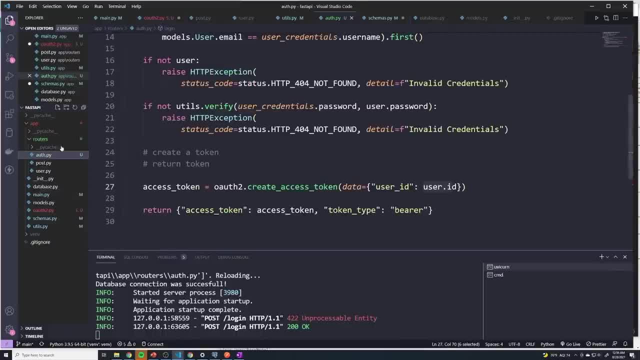 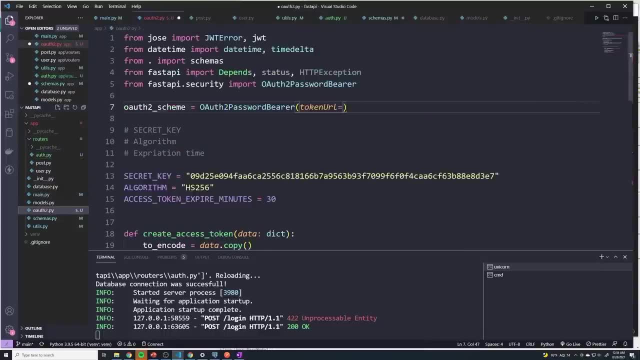 of our- basically our- login endpoint, And so if you go to your author py, you just grab whatever name this is. Keep in mind, you don't have to name it login, but you just have to pass this into here. Actually, sorry, you remove the slash, So it's just login. 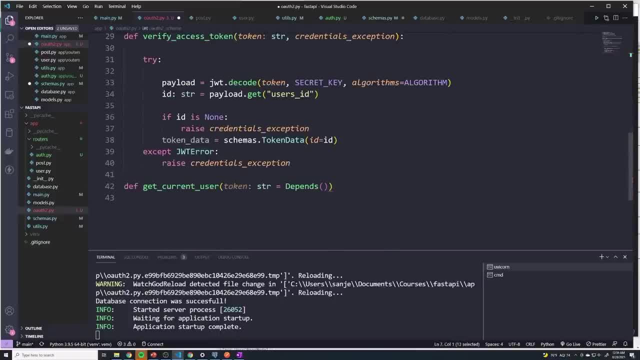 And then we're going to grab this variable And I'm just going to pass it into here- And this is kind of just tying everything together- And then we have to define our credentials exception that we're going to pass into the verify access token function. So when the credentials wrong or there's some kind of 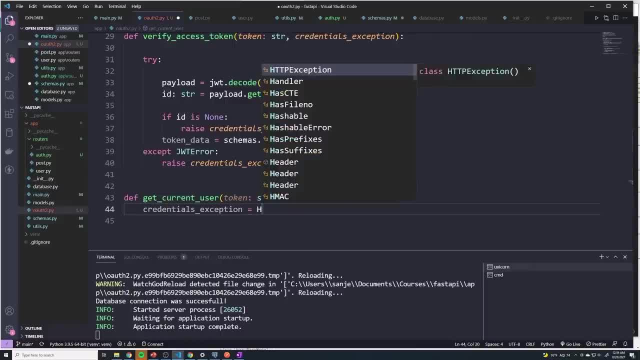 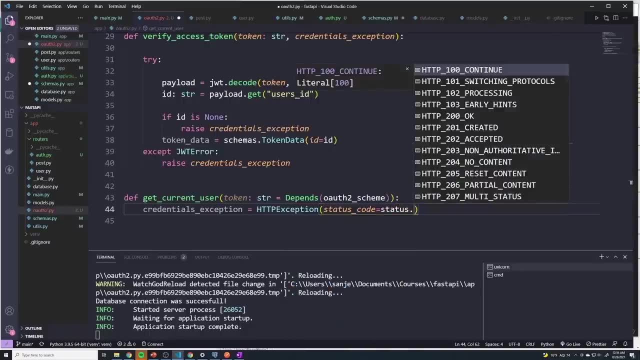 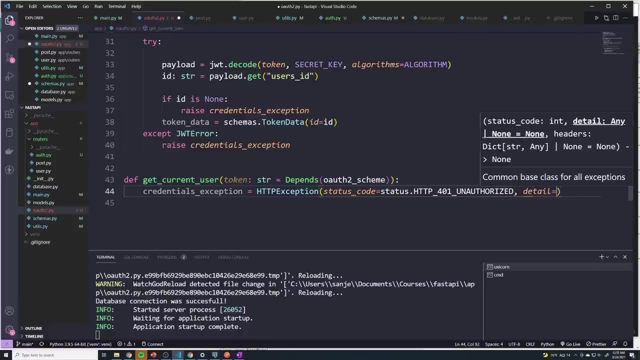 issue with the JWT token. what exception should we raise? So here I'm just going to say HTTP exception And we'll set the status code to be a 401.. So unauthorized detail. I hear I'm going to pass a string Once again. could not validate credentials. 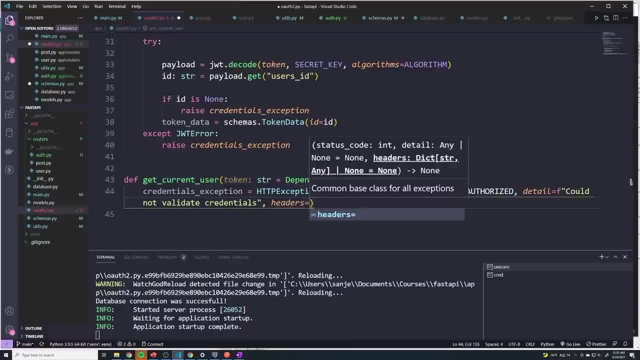 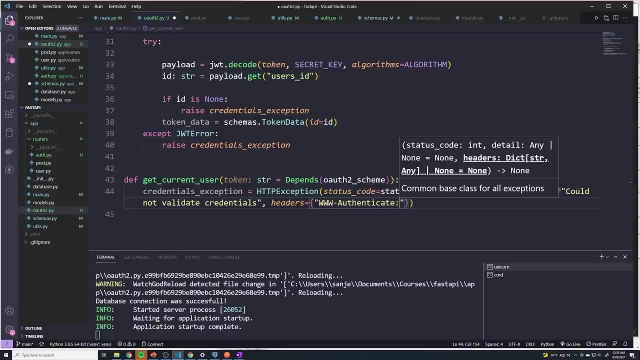 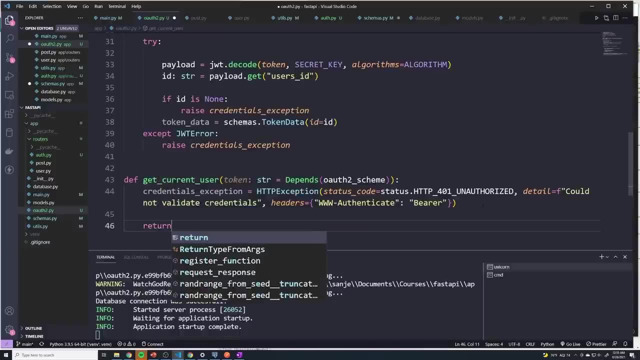 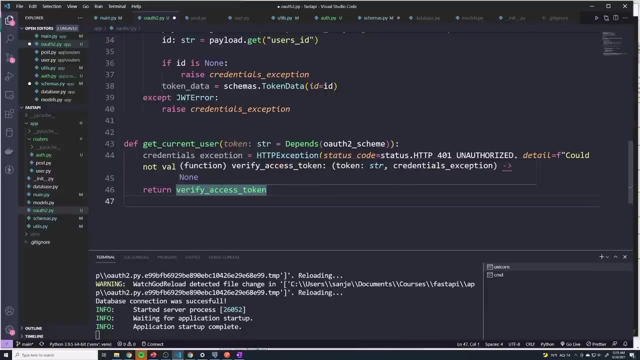 And then we have to set some headers as well, And so just go ahead and just copy this in, And then, finally, we're going to return a call to our verify access token function, And since we have the token pass into the Get current user, we can pass it into our 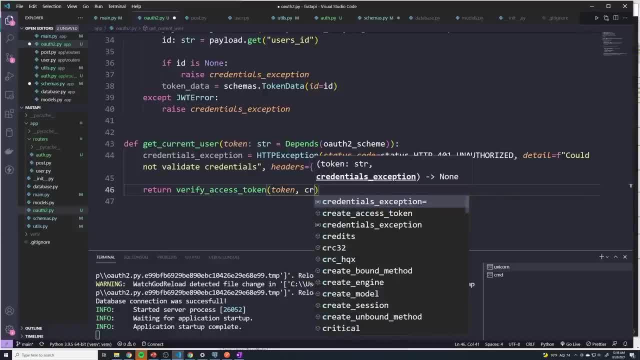 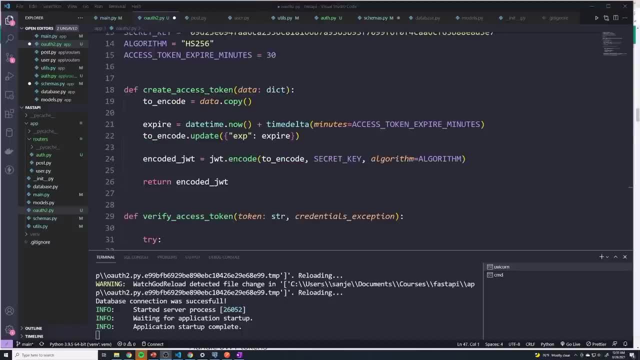 verify access token And then we also can provide the credentials. Alright, so just to quickly recap, because I know we did a lot and I think some of it may be confusing: We do this from the source command right, But what's going to happen is, anytime we do that, we're going to save this. 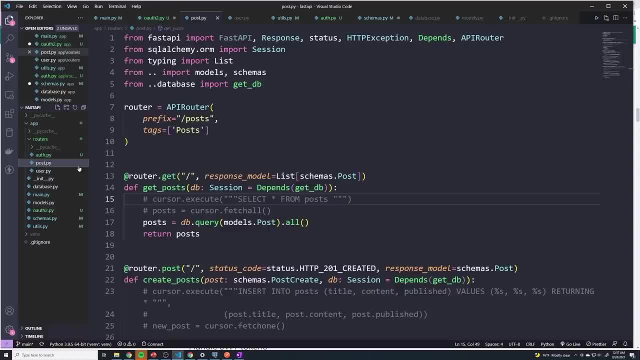 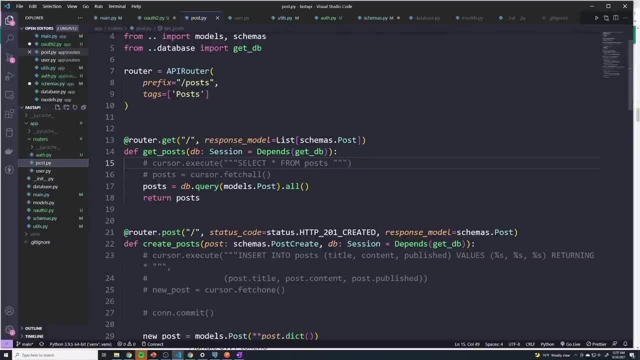 happen is anytime. we have a specific endpoint that should be protected, and what that means is that the user needs to be logged in to use it. what we're going to do is- I'm going to well, as an example, let's say that users who want to be able to create a post, they 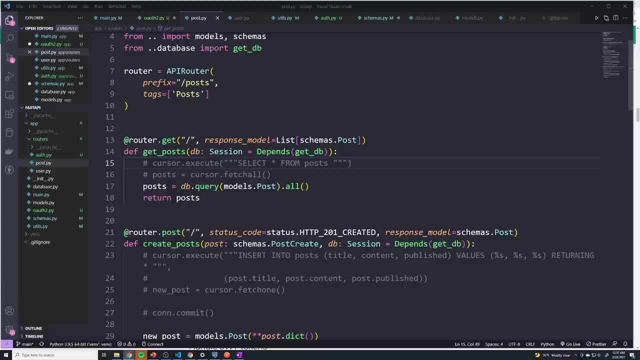 need to be logged in. what we can do is we can just add in an extra dependency into the path operation function. So I can say here I would just say: get current underscore user, which would return an int, And then we'll say this equals, and then we pass in a dependency. 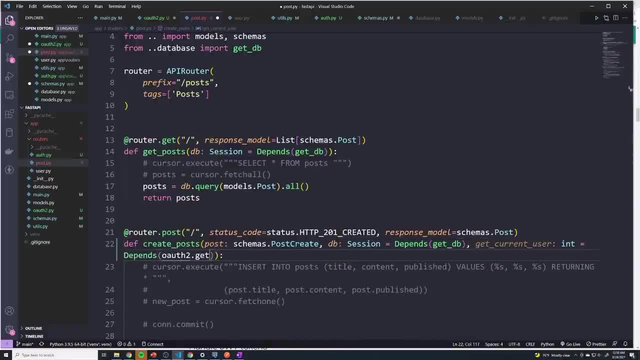 So we'll say: depends on a lot to dot get underscore current user. So this is going to add a dependency, which is going to be that function that we created called get current user. So anytime anyone wants to access a resource that requires them to be logged in, we're going to expect. 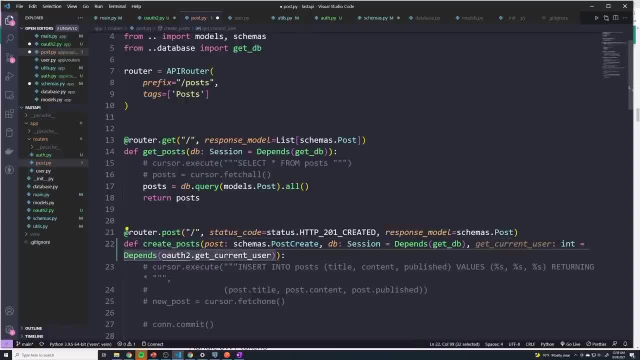 that they provide an access token. And then we provide this dependency which is going to call this function, get current user. And then we're going to add a dependency which is going to say: get current- sorry, where is it? get current user. And then we pass in. 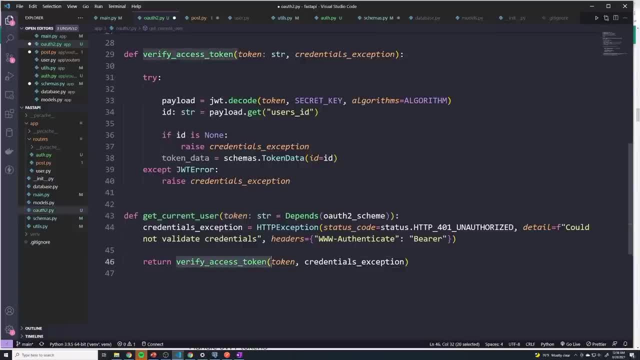 the token that comes from the request. we're going to then run this verify access token in this case, And then it's going to provide all of the logic for verifying that the token is okay and that there's no errors. And if there's no errors, then we go ahead and return. 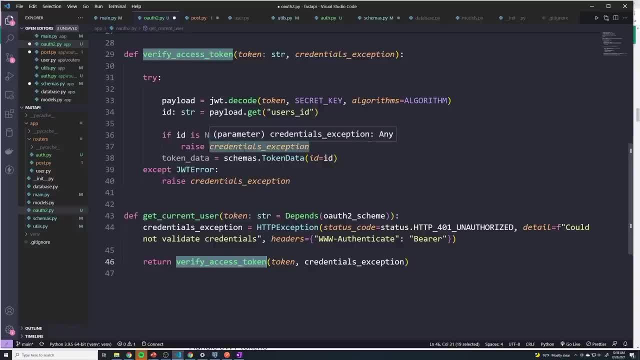 nothing essentially, And that means that they were successfully able to be authenticated. If we do return some kind of error with the credentials exception, then they're going to get that appropriate 401 response back. So that's how our login works. It's nothing special, But there are a couple of different. 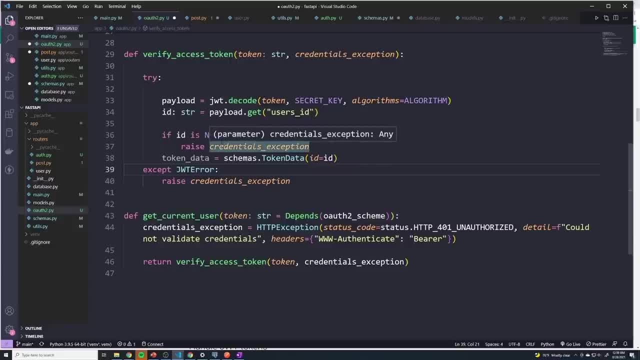 components that are involved And in the next lecture we'll start to take a look at starting to protect our specific endpoint so that it forces users to be logged in to actually perform that operation. And guys, I made one little mistake In the verify access token function. 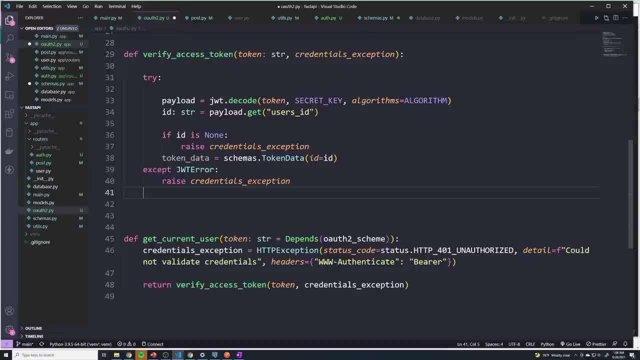 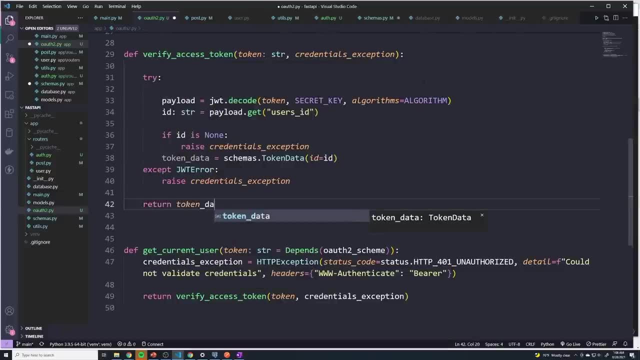 I forgot to return something, And so if you ran into any issues, it's because of this. So what we're going to do is here is we're just going to do return token underscore data, And so what's really happening here is, once again, we're going. 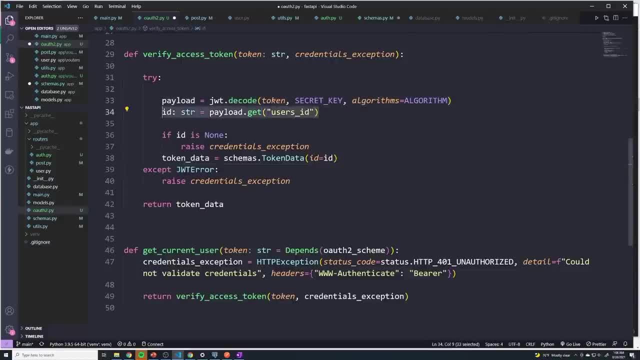 to decode the JWT, we're going to extract the ID. If there's no ID, then we're going to throw an error And then we're going to validate with a schema of the actual token data, which in this case is just an ID. So that's the only field. but if you had extra 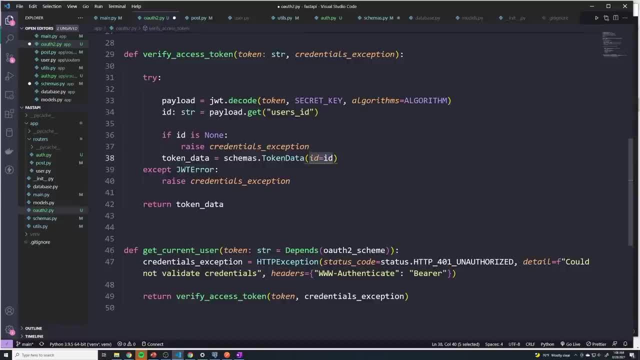 properties are extra information. you can pass that in. And then we want to make sure that we return the token data so that we can actually make use of that data. otherwise there is no problem. Then we want to put out an update to this data, And then we're going. 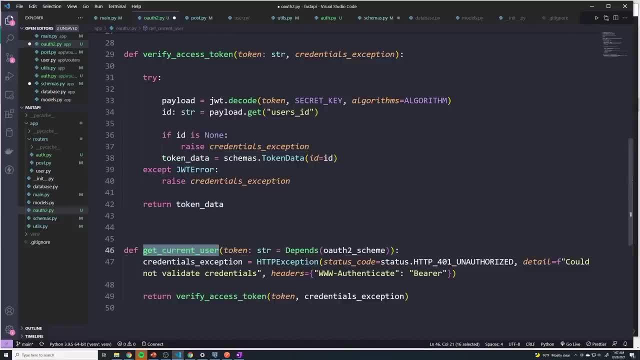 to that data And keep in mind, remember the get current user is what actually calls the verify access token. So when it calls verify access token, it expects us to return the token data And then, when we get the token data, we return it to whoever calls this function. 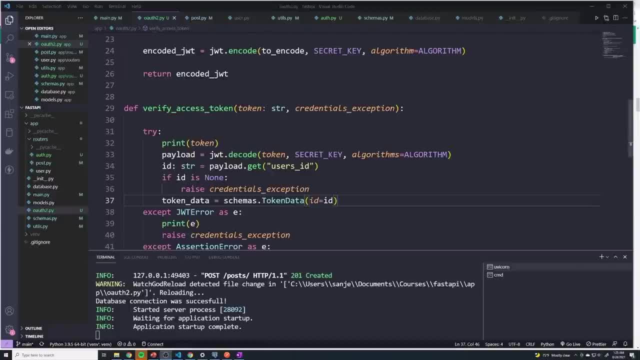 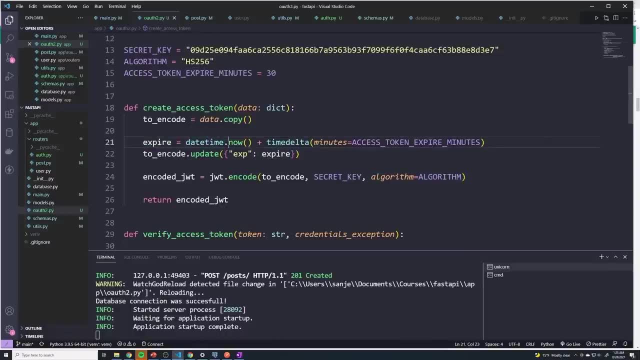 Okay, guys, so I found a few extra bugs that we need to fix. Now, the first thing that I messed up was when we actually set the expiration time under the create access token function. instead of datetimenow, it should be datetimeutc. now, This is important because, as I was testing it, 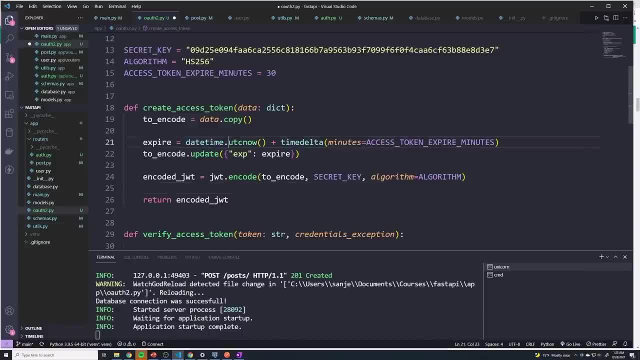 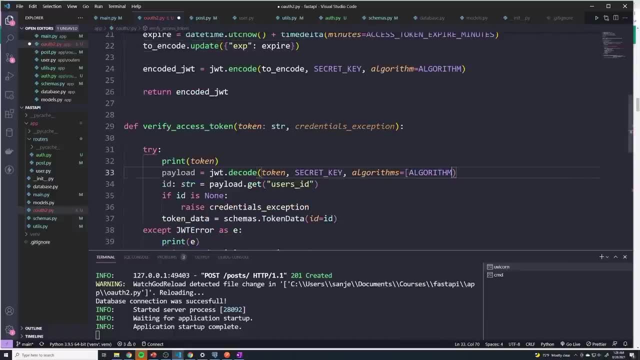 I kept getting an expiration error, And that's because this should be a UTC Now. And the second thing is, we want to put this in brackets because I guess it expects a list of algorithms. maybe we'll put that in there. And then, finally, this is also a bug right here, Because if you take a 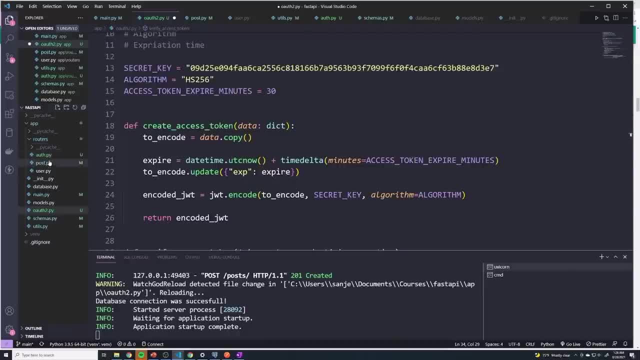 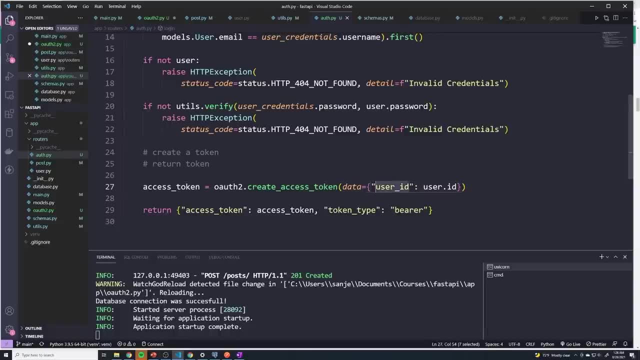 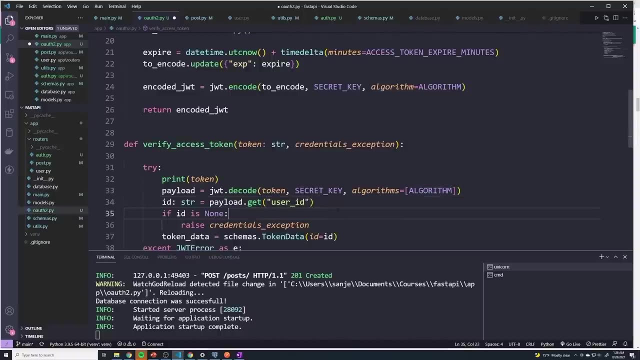 look at the payload when we create the token, which I believe should be in the authpy, When we log in, we pass in the data as user underscore ID and not users underscore ID like we did here. So remove that And this should prevent us from running into any. 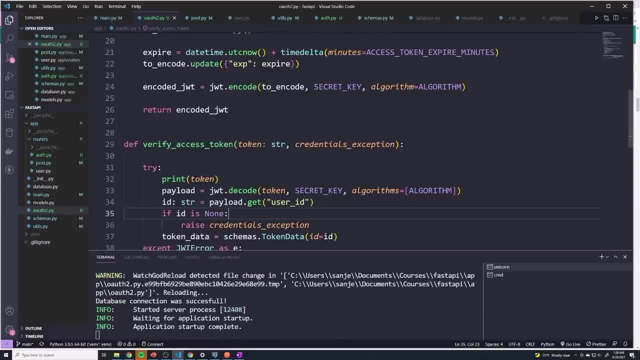 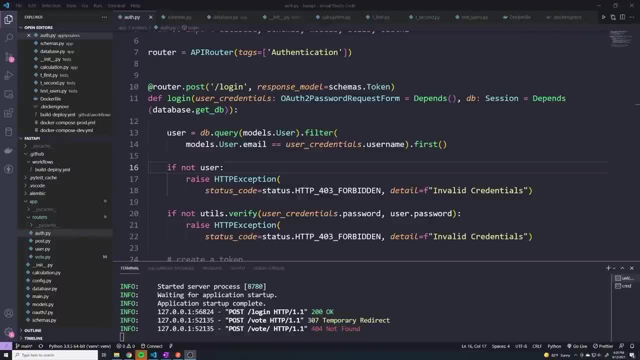 other potential issues in the upcoming lectures. Sorry about that. I know we ran into a couple of bugs, But that's what happens when you try and copy and paste really quickly. Before we wrap things up, there's one last change that I want to make inside the login route in the authpy router. 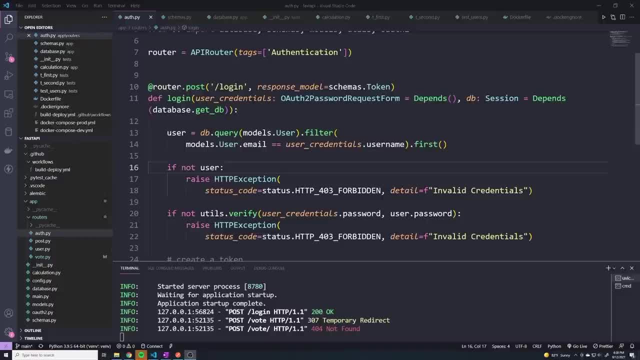 file. I noticed that for the response or the exception that we raise, if the either the user's email is wrong, or if the user's email is wrong, or if the user's email is wrong or if the user's password is incorrect, I use the wrong HTTP status code for the exception And I can't remember. 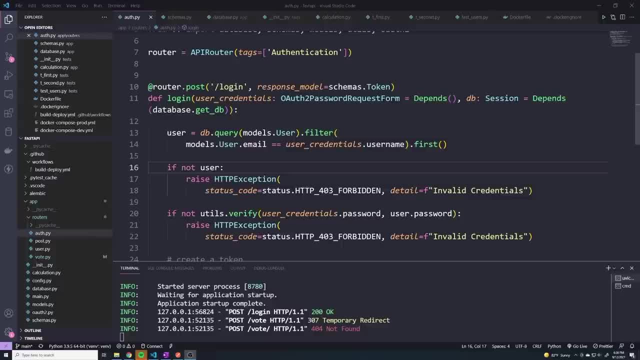 what I actually had it before, because I went ahead and fixed it. But I want you guys to go ahead and change the two exceptions here In both of those cases to a 403.. I think that's a better representation of what we should be sending when the user doesn't provide proper credentials. So 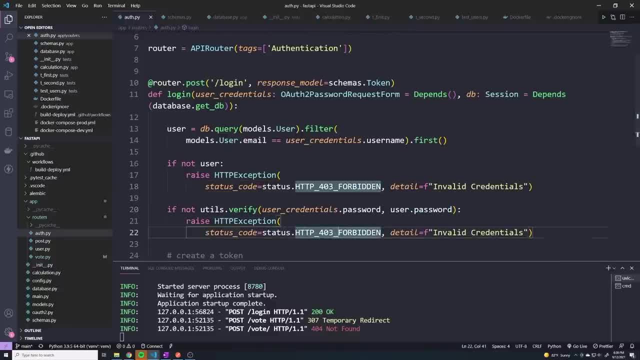 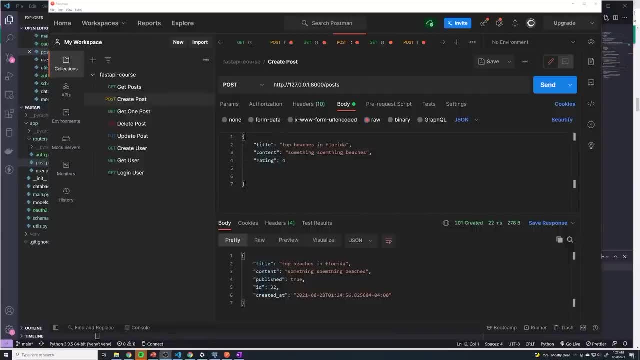 just update it here, and then update it here as well, And then you guys should be good to go. Okay, guys, we're pretty much done with all of the authentication side of things. The only thing that we have to do is require the user to authenticate, because right now you know, 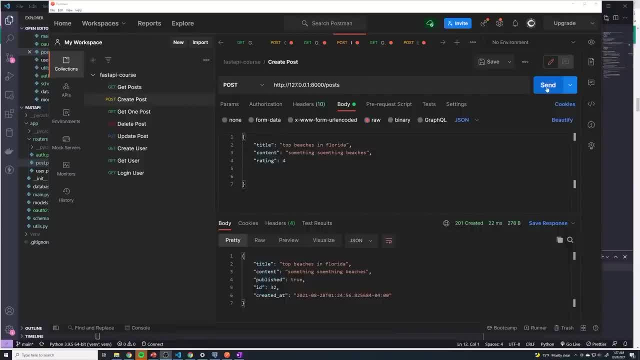 if we perform any operation like creating a post, you can see that I could just create a post And that's it. I don't have to log in first, I don't have to do anything. So anyone can create posts, anyone can delete posts, anyone can do anything they want. Obviously, that's not how. 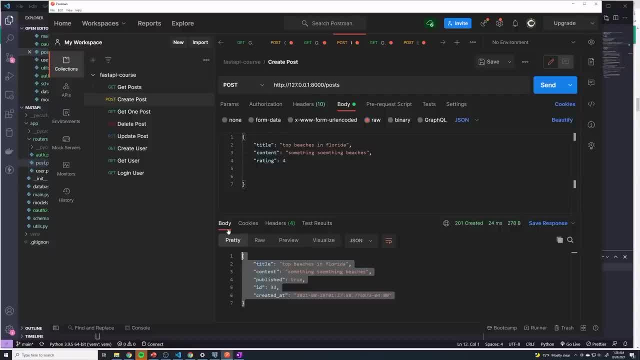 your API is going to work. You're going to want to ensure that users are logged in to perform certain operations, And there may be certain operations where they don't necessarily need to be logged in, depending on how you're using it, So I'm going to go ahead and change that. 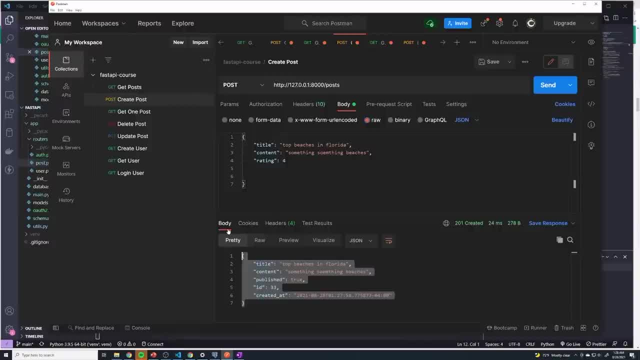 How you want to structure your application right, Because you know, if it's like a Twitter, like application, right, anyone can see anyone's tweets. I just can't delete anyone else's tweets, right, And to create a tweet, I have to be logged in, And so it depends on what you want to do for. 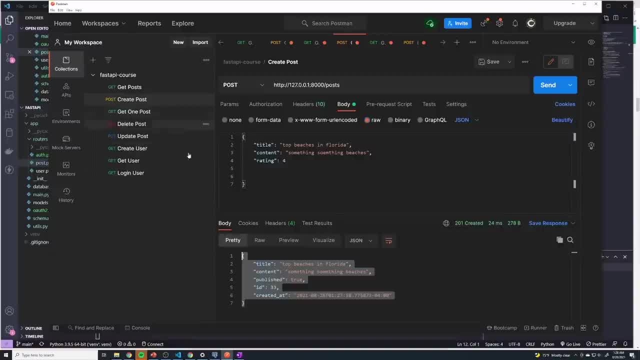 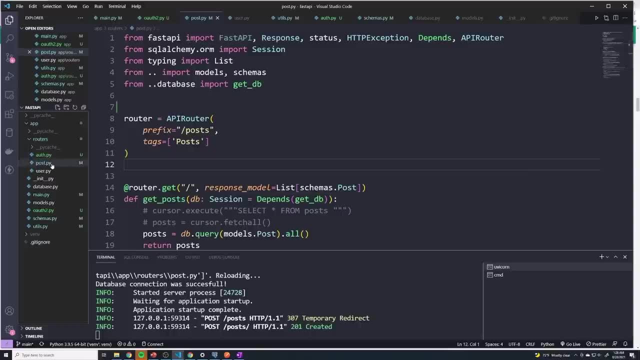 your application. But what we're going to do is we're going to start off by forcing the user to be logged in before they can create a post, And doing this is actually really simple. So let's go to our postpy And let's find our create posts. Now, the first thing I want to do, 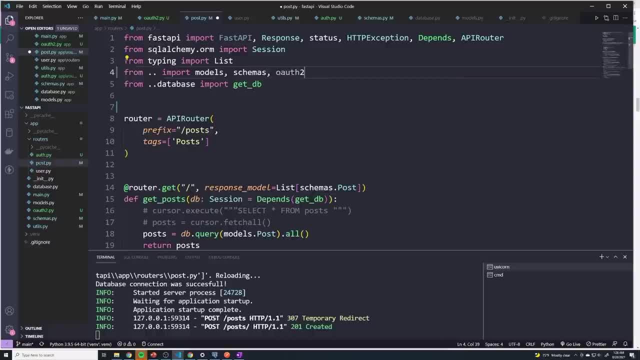 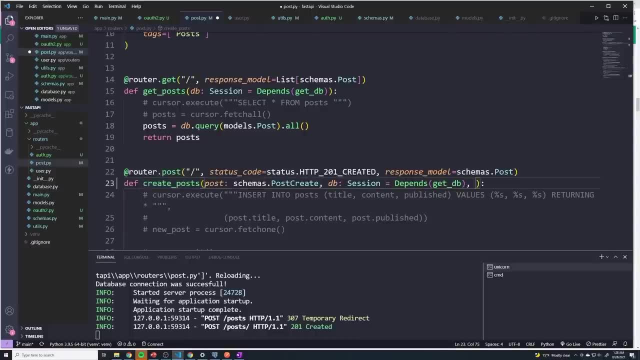 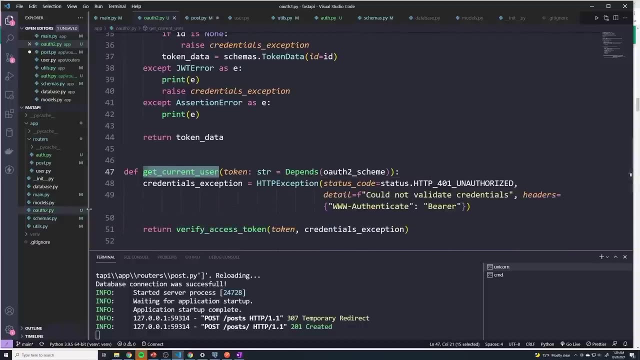 is. I'm going to import a lot to which is coming from this OAuth2.py file, And then, in our create posts path operation function, we're going to add an extra dependency, And this dependency is going to be the create- or, sorry, get- current user function that we defined in our OAuth2 file. 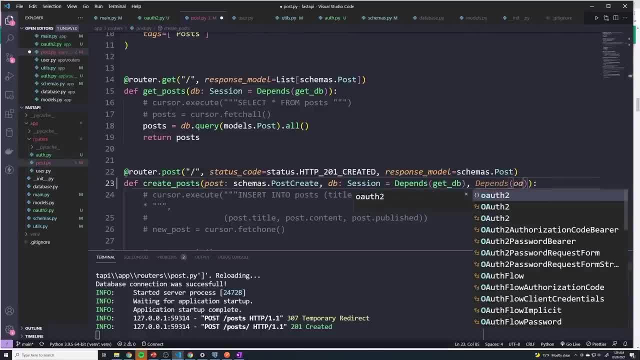 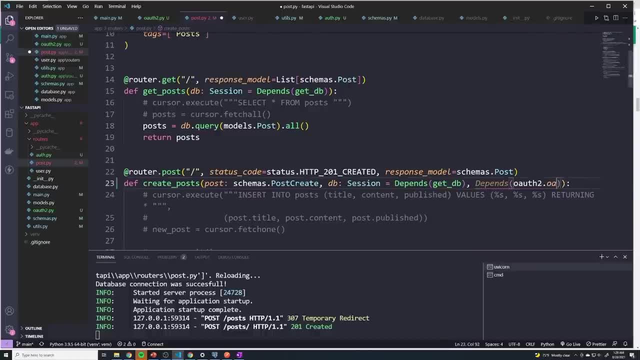 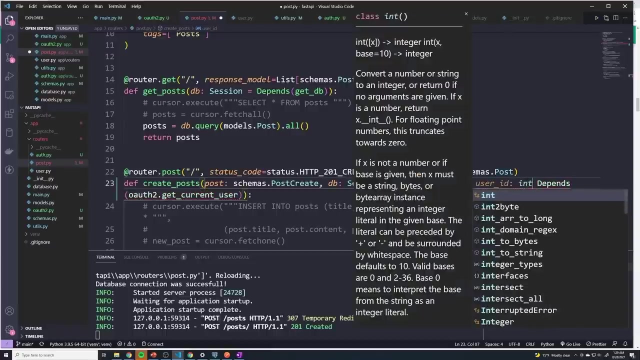 So we'll say is depends. And then we'll say OAuth2.get underscore current user, And then we're going to store this in a variable called, let's say, user, underscore ID, And this is going to be a integer. Okay, and so all this is saying is that this function is now. 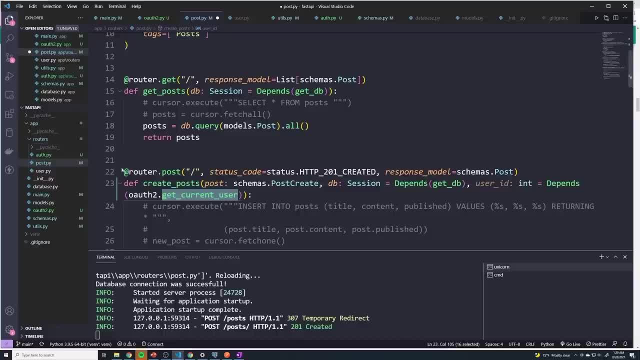 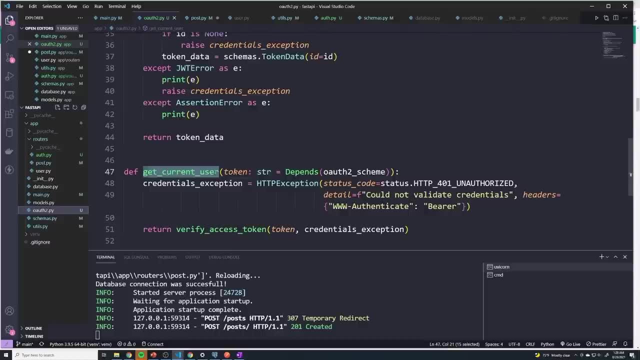 going to be a dependency. So this is what forces the users to have to be logged in before they can actually create a post, And so when this function is called, whenever they hit this endpoint, the first thing that we're going to do is we're going to call this function And this function. 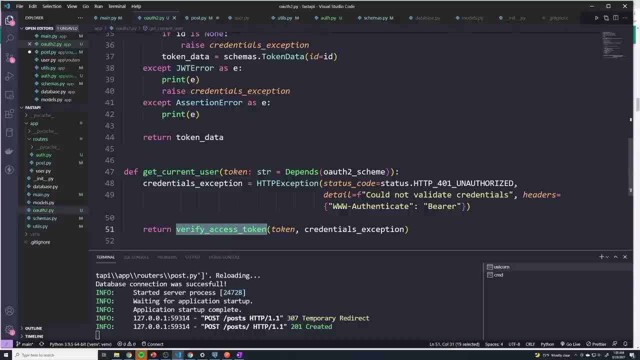 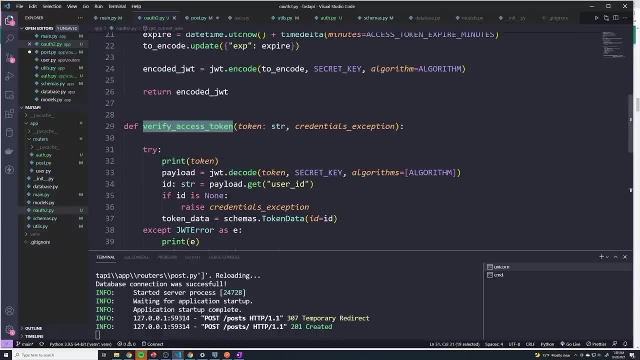 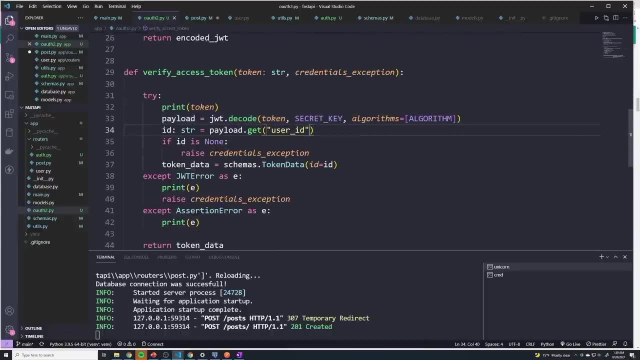 all this function does is really just call the verify access token but and passing in the tag in the token which comes from the user, And so it takes the token, we first decode the token, we extract the ID from the payload And if there's no ID we throw an error And then you can see we. 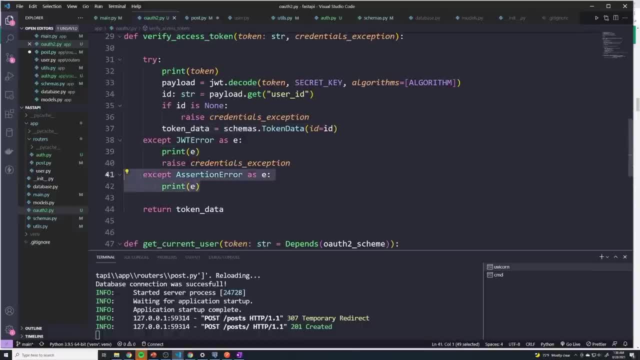 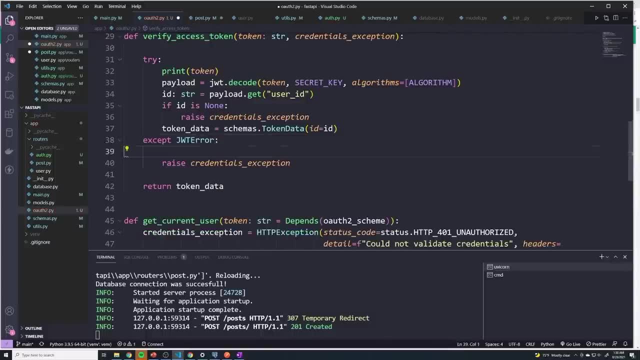 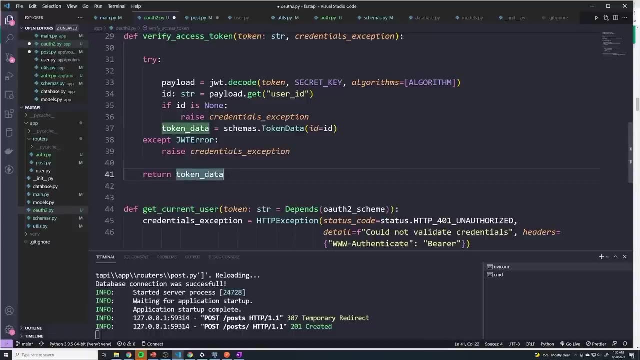 validate the schema And then this side. this is something I actually added in off camera, So we can just delete that And then go back to what you guys have. But we ultimately return the token data, which is nothing more than the ID. Right, So we could rename this as ID for now, But, like I said, in the future 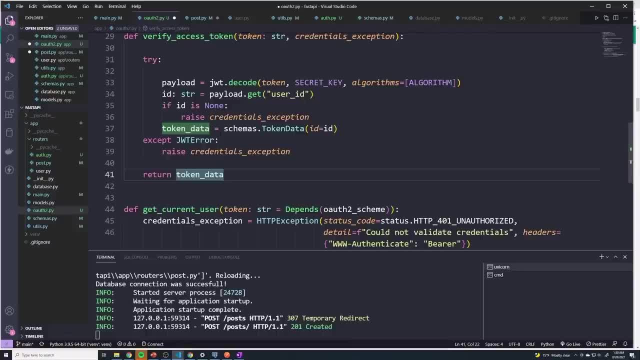 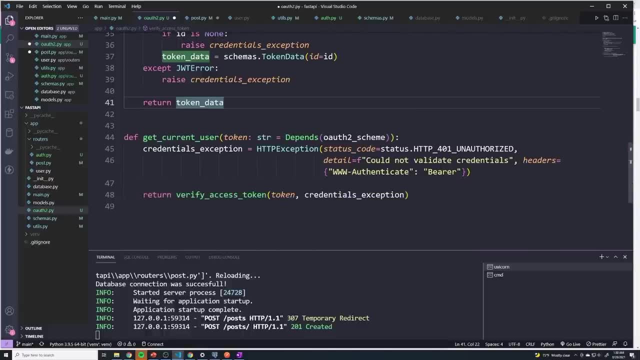 you may want to add extra fields into the payload And then it's no longer just the ID, it's going to include extra information. So we're going to return the ID, which then gets returned by the get current user function, And then in our post up py, in our function, we're going to return the ID and stored. 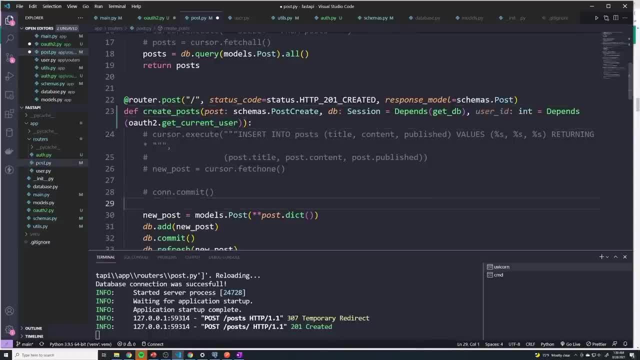 in a variable called user ID, And so then we can ultimately access the user ID by just calling user underscore ID. That's it, And we can do whatever we want with this user ID. And you'll see, we'll eventually add some more logic, But for now I'm just going to print it out, just to see. 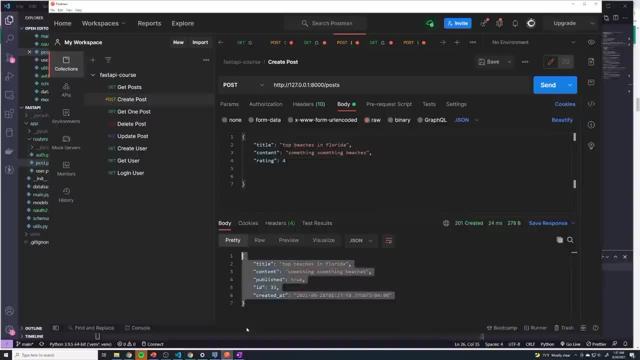 what we see, And let's go ahead and try this. So first of all, I'm going to create post And then we're going to see what happens. now, when I try to create a post, Look at that: not authenticated. So by putting in that extra dependency, we have ensured that the user has to be authenticated. 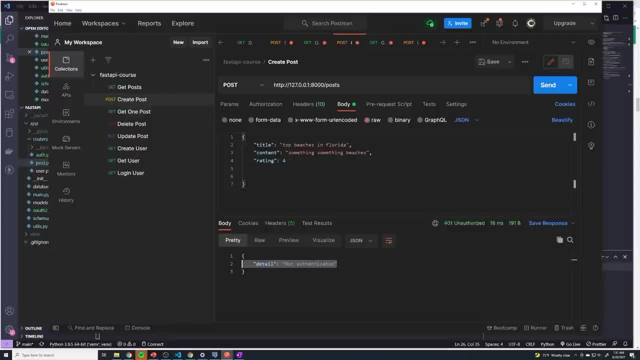 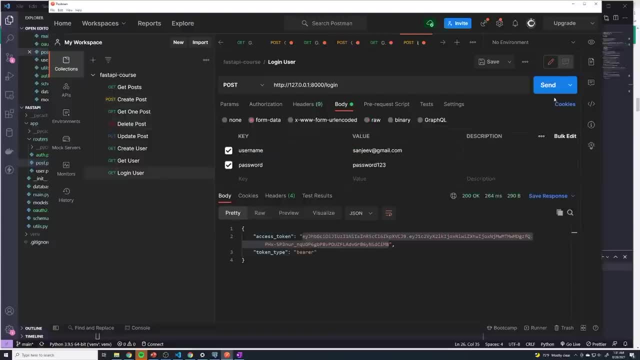 before they can use this post. Now, how do we actually provide the token so that we can actually use the create post? Well, first of all, let's get a token. So we're going to go to the login user. I'm going to hit send. 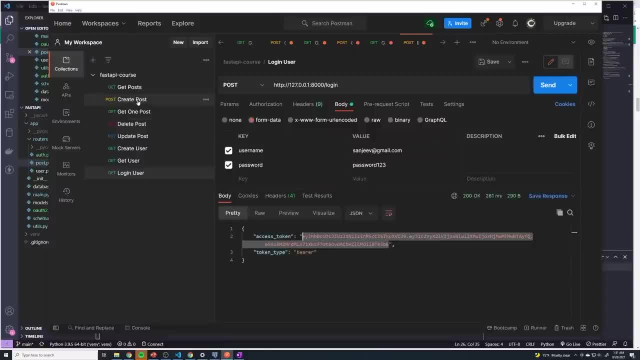 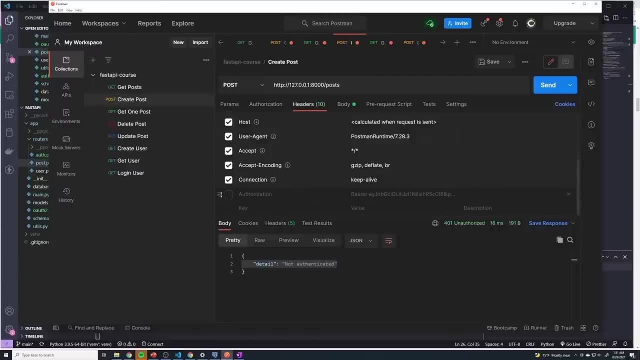 And get a brand new token. And then what we want to do is we want to go to create post, And then we want to go do headers, And then we want to create a header. And you know, you can see, I can. I created one already, But I'm going to type this out for you from scratch in the line below it. 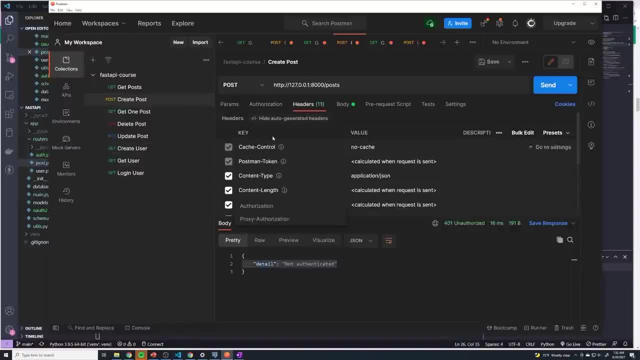 So we say authorization is going to be the, the key, And then the column is going to be, and you type the word in bearer, because it's a bearer type token. So you do bear with a capital B space. don't forget the space. 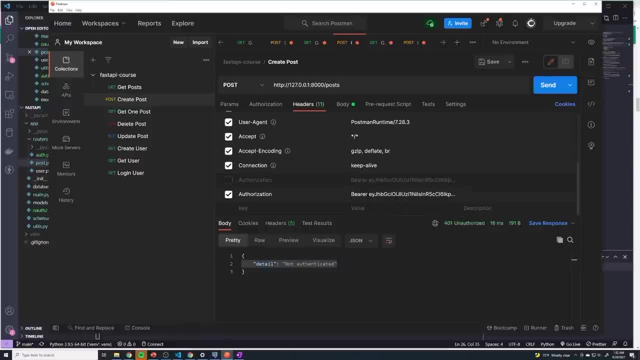 And then paste it in. Okay, and so now this is included in our header, And so we should be able to send a request. And so now, look at this- we were now successfully able to send our token. the API was able to validate it was a valid token, And it was able to then allow us to create a post, And 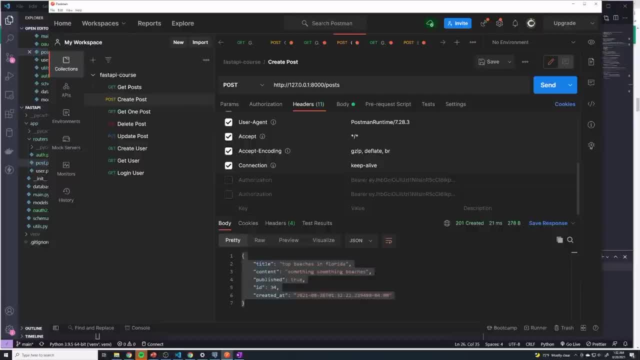 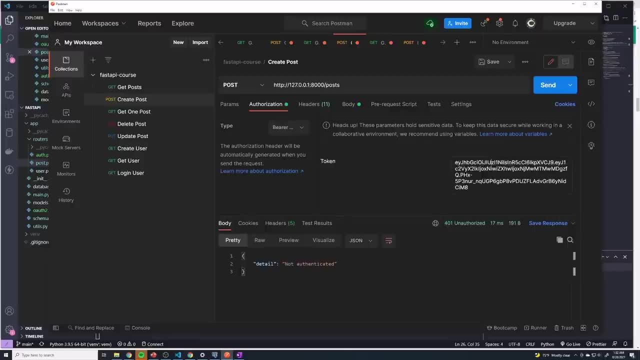 just another little postman tip. you can uncheck this for now. So that is not authorized. See, if I try to do it now, you see I get it And then you can go into authorization and then just type in, go to bearer token and then paste it into here. does the same exact thing. It just you don't have to type in the word bearer for yourself And then you know, have to do all of that. you could just hit send now And it does. does the same exact thing. whichever method you prefer more. 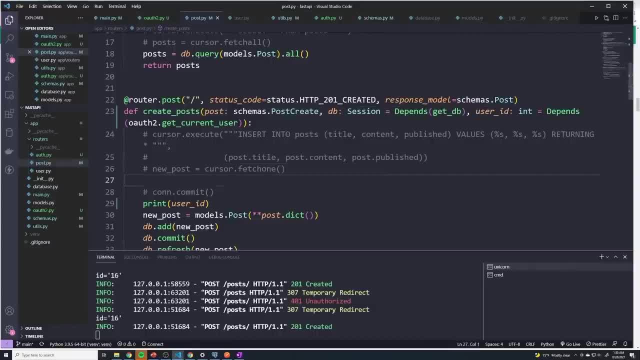 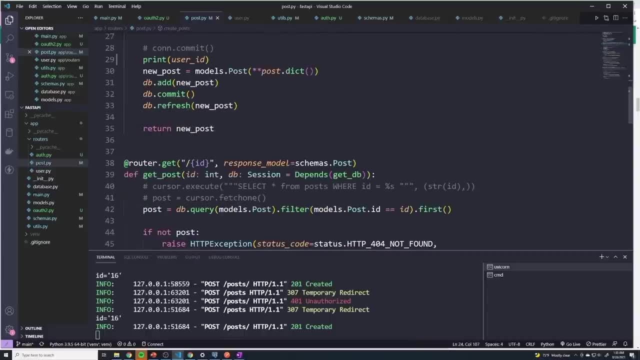 Now that we've protected our create posts route, let's go ahead and do this with some of our other routes. So it's just a matter of just copying the dependency for get current user and then for retrieving a post. Well, remember, this part is up to you. you decide ultimately what. 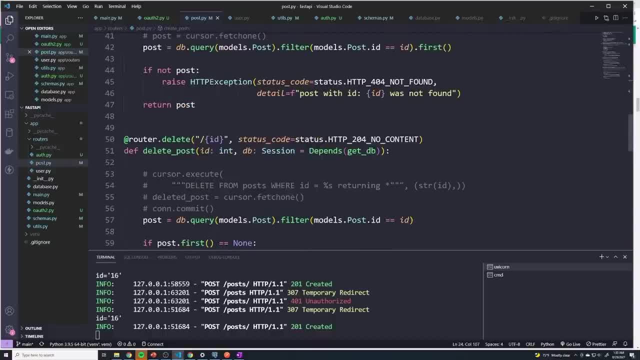 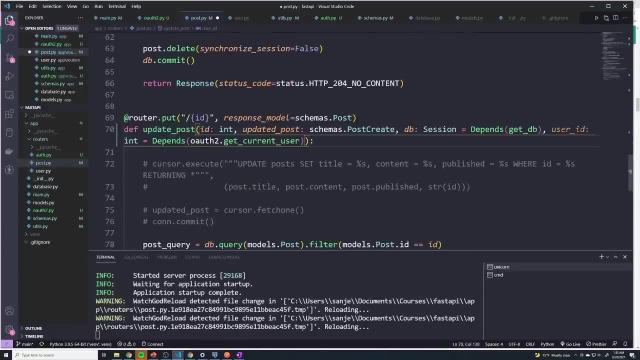 routes. you want a user to be logged into, actually perform an operation. But for delete posts, I'm definitely going to force a user to be logged in, And for update Post, I'm gonna do the same thing, And then, finally, you know, like I said, forgetting posts. you know it's really up to you, we'll see that. 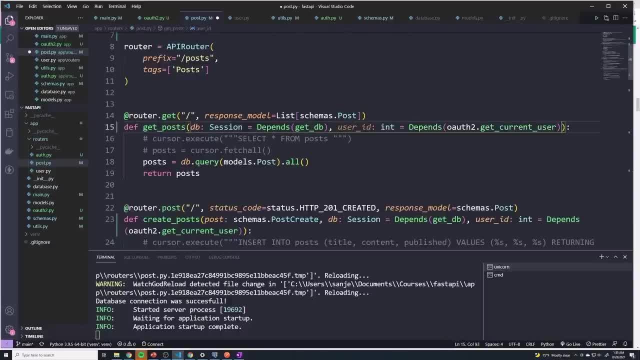 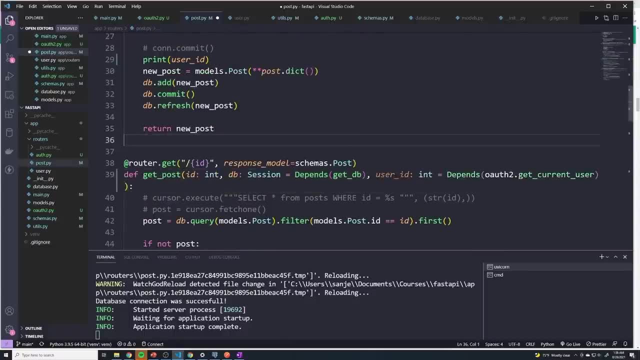 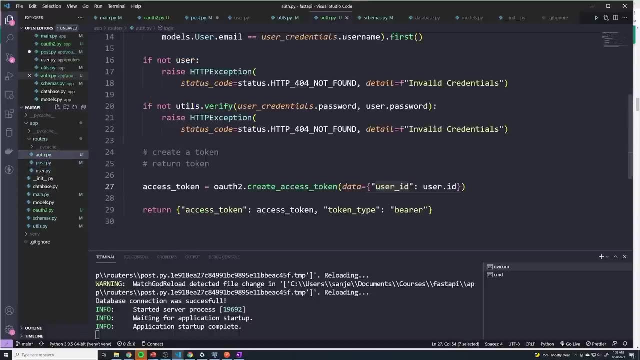 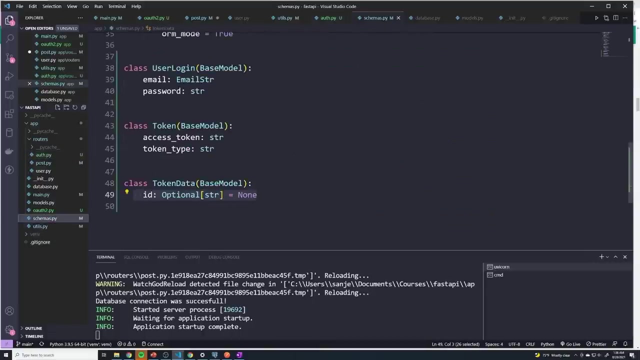 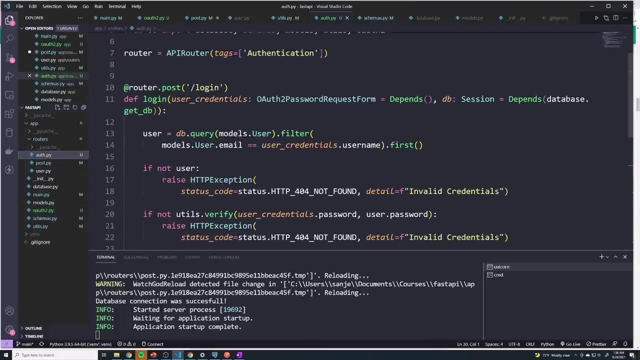 you have to be logged in to do anything. So forget posts are getting all posts. we want to make sure that are logged in. And then, forgetting an individual post: we want to make sure that they're logged in. And then, finally, the last thing that we- well, it's not the last thing, But one of the things I forgot to do is under authpy, When we send our access token after they log in. if you remember, in under schemas, we actually created a token model, or, sorry, token schema. we never actually used it. So let's actually use that by setting the response model here. 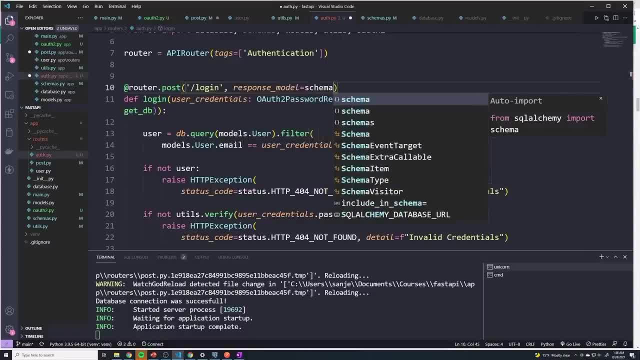 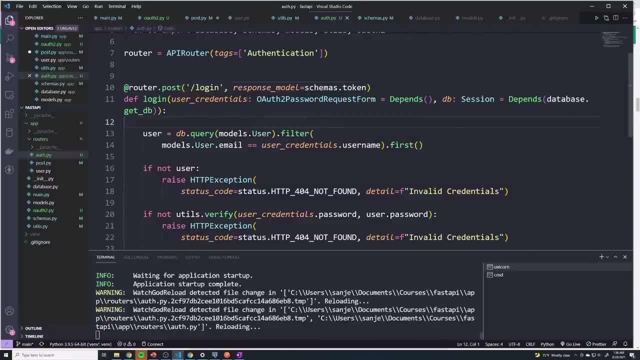 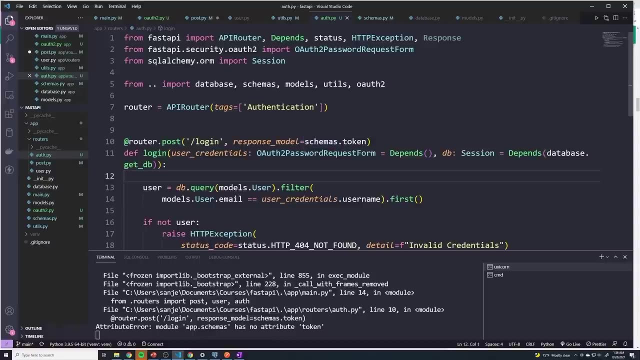 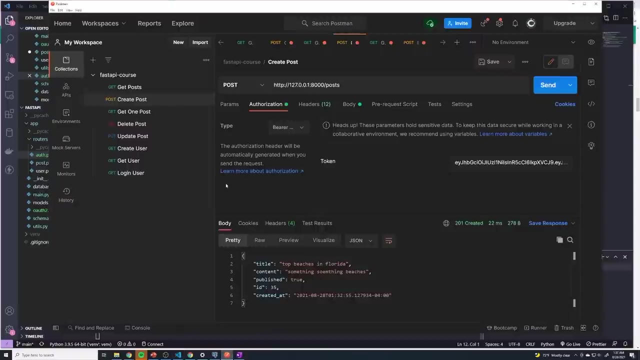 And this is going to be schematoken, Schemastoken. Let's save this And this should be capitalized. Sorry about that. And so now, if we log in a user, we should still get no error, So perfect, Okay, so just in case in the future, 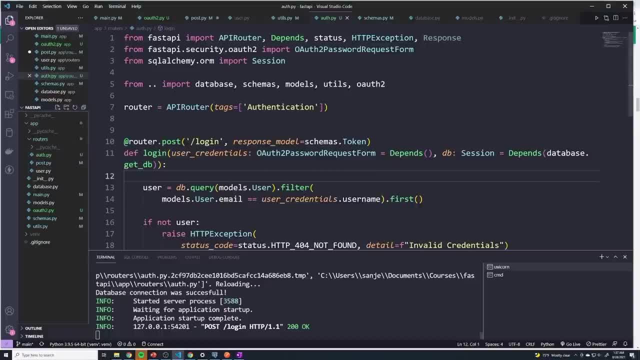 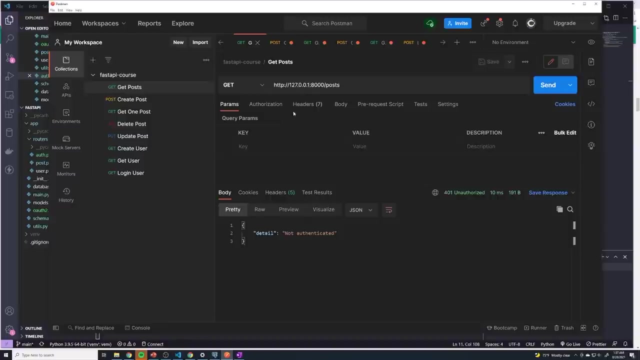 we accidentally change something. we're still going to perform that validation to ensure that the token we only send those two fields when we return a token. Now let's quickly just test all the other routes. So if I do get posts and I hit send, you can see: well, let me save everything. Sorry about that. Once again Now if I hit send, you can see I'm not authenticated, So I have to do the same thing. So once again you can do authorization bearer or you can go to authorization and then just 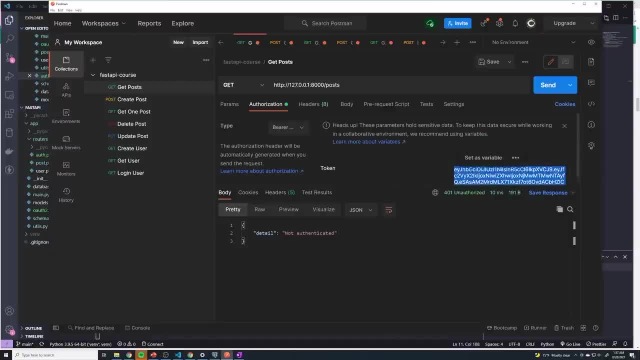 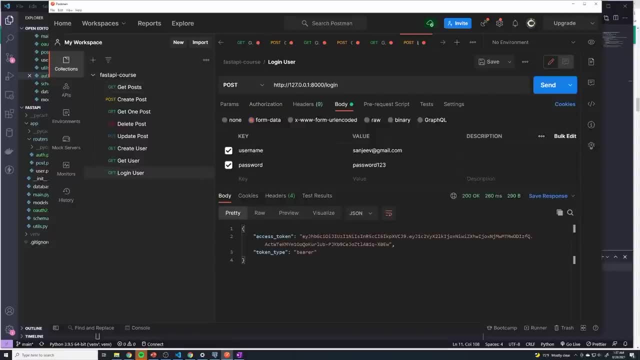 select bearer token and then paste in the token. Now if I hit send- oh sorry, I got to recopy the token again. Now- if we send, it works. now get one post. let's try this. not authenticated, we'll go into authorization. Bearer token: Send. that works deleting posts. Go to once again to authorization. 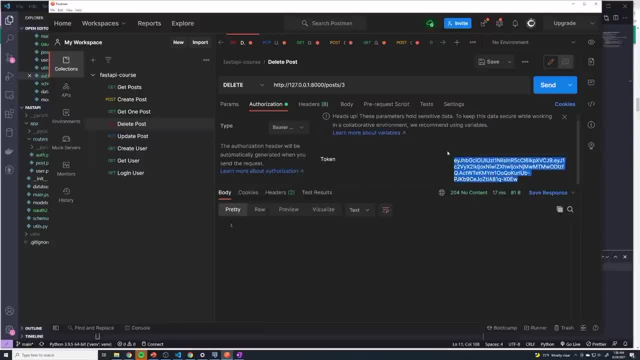 And there's no post with an ID of three, about four, All right, that worked. And then finally update post. We're going to do the last thing and bearer token- All right, and that works. And then let's just double check to make sure that, if there's no token, what happens? Error Perfect. Okay, guys. so I think that's going to. 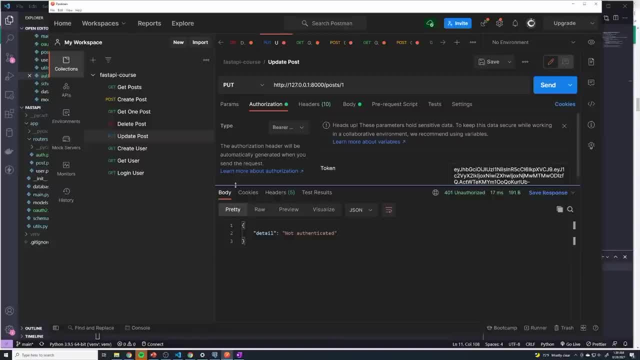 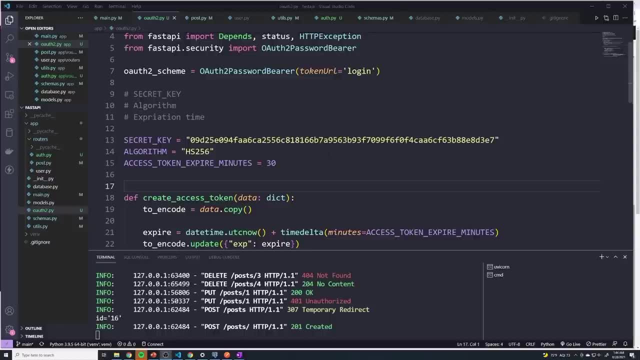 wrap up this video. for now, we've pretty much done all the authentication that we need to do up to this point. There's one last thing that I want to test to verify that everything works the way it should- And we probably should test this in one of the previous videos, but I forgot to do it- And I want to make sure that we test the expiration process, because a JWT has an expiration time that we set ourselves, And this just ensures that a user is logged in only for a certain amount of time. Now we set the access token expiration time to be 30 minutes. 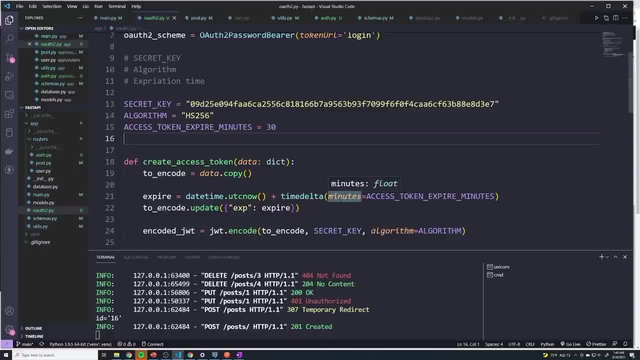 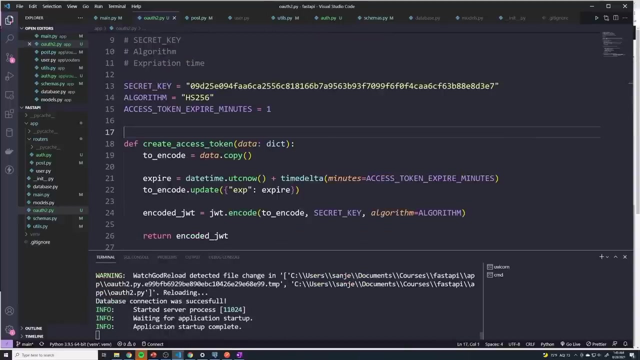 And so that means that if a user logs in and he keeps his token for more than 30 minutes after that 30 minute mark, if he tries to use that token to access any of our endpoints, it should throw an error because it's already expired. So let's test this out, And the easiest way to test this is, first of all, we're not going to wait 30 minutes. That's ridiculous. So what we're going to do is we're going to set this to one minute And we're just going to test this real quick, And so I'm going to log in this user. 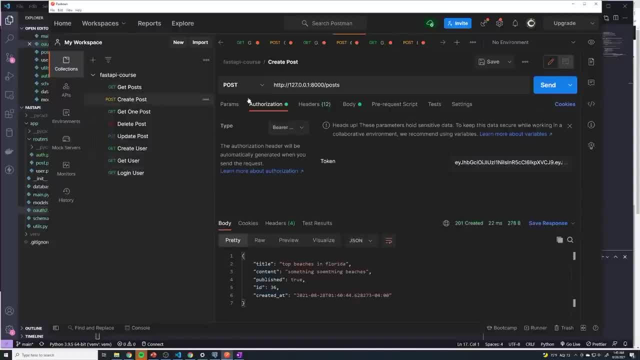 This token is valid for exactly one minute, And so we'll go to create posts- actually, we'll just do get posts, it doesn't really matter- And I'll paste this in here And you'll see this works. And we're going to just wait for one full minute And after one minute let's just verify that we get a unauthorized error because the token has expired. Okay, so it should be about one minute now, And so if we test this, we should now get an error. So after one minute it says it could not validate credentials, that we could set up a log message to say that, hey, this token is expired. 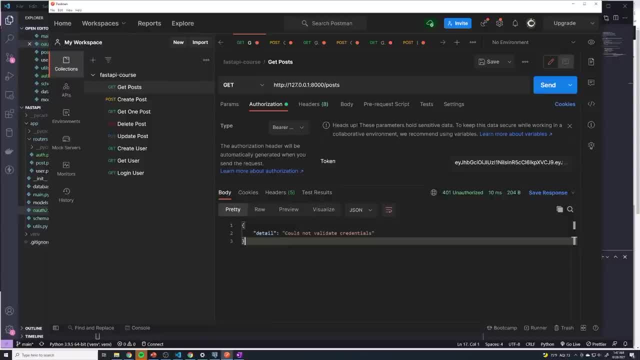 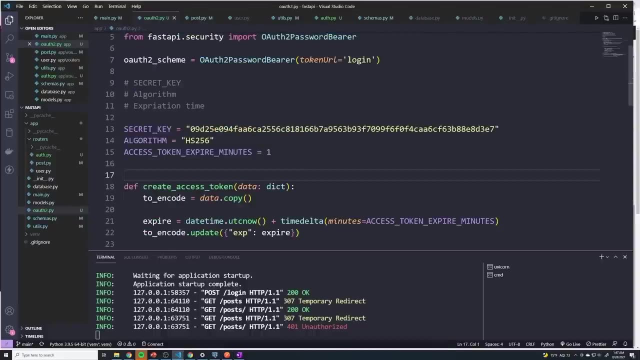 But we don't need to worry too much about that, As long as it throws an error and it gives them a 401.. I think that's good enough for now, And so this confirms that our expiration functionality works, And the last thing to do is: well, let's make sure we change this back. So, once again, it doesn't matter what time you choose, it's up to you. I'm just going to do 30 minutes. Actually, I'm going to do 60 minutes just for testing purposes. Moving forward, I don't want to have to continually get a new token after every 30 minutes. 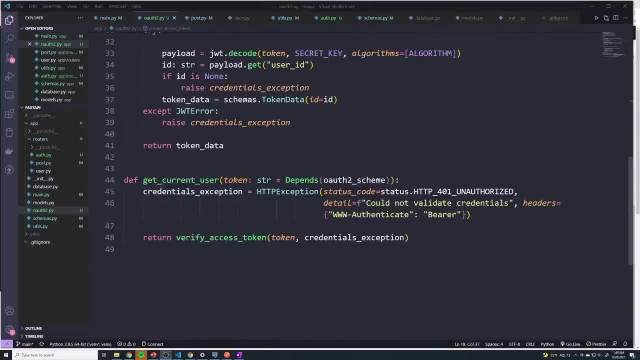 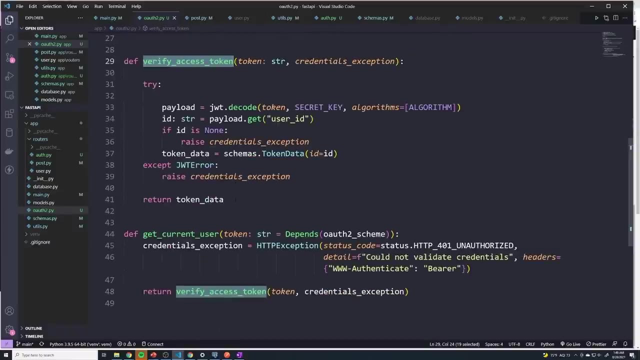 So 60 minutes is a good number. Now you might be wondering why exactly do we have this get current user function when all it really does is just call verify access token. we could completely just remove this and just call this directly whenever we want to authenticate a user, And you absolutely could with the current implementation. But the idea behind the get current user function is that once the verify access token returns the token data, which is the ID, the 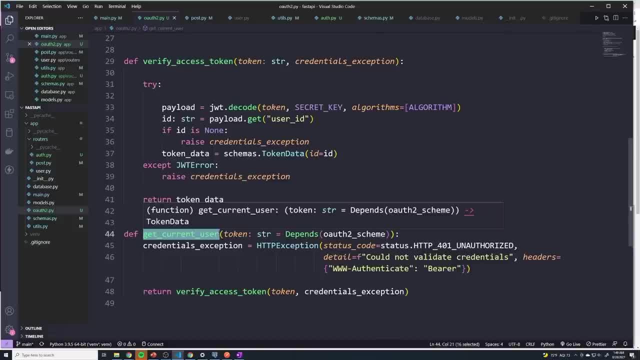 get current user function should actually fetch the user from the database, And so that way, we can attach the user to any path operation and then we can perform any necessary logic. Now you don't actually have to fetch the user here. It's up to you how you want to implement this. If you want each of your path operations to fetch the user themselves, they have the ID so they can do it themselves. However, if you wanted to automatically do it here, you 100% can do that, And so I'm going to show you guys how you can do that in this lesson. And so keep in mind, we get the token data back. 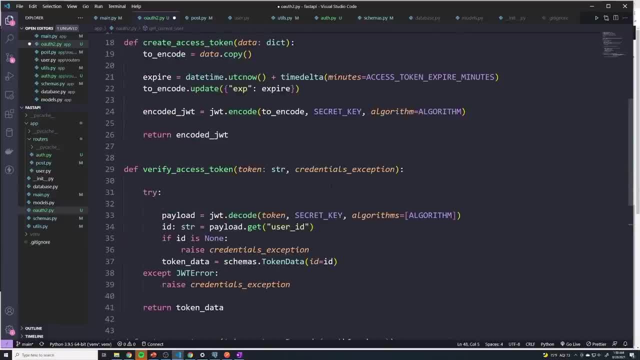 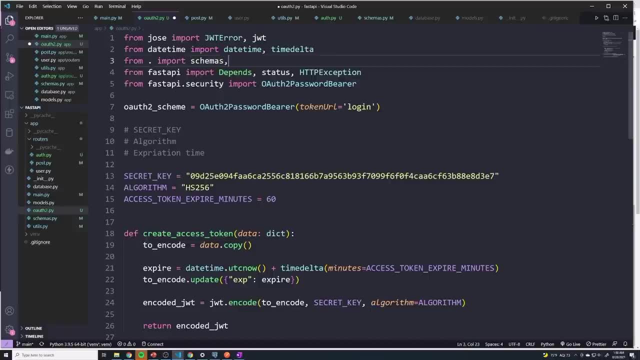 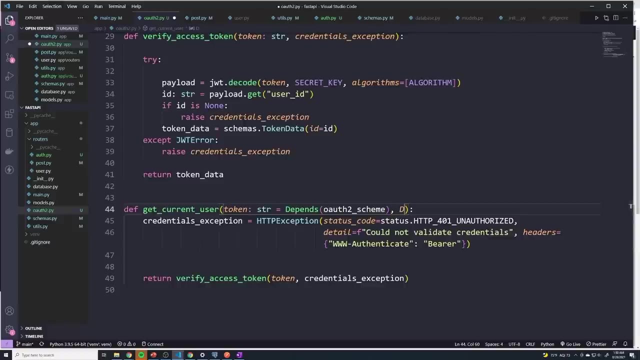 which is going to be nothing more than an ID, And what we're going to do is, first of all, we need access to our database so that we can fetch the users. So from here I'm going to import database And within this function we can pass in the, the dependency, so that we can actually get access to the DB object. So I'll say depends, And then we're going to access database dot, And I already forgot the name of the function. What does it get? underscore DB? I'll get 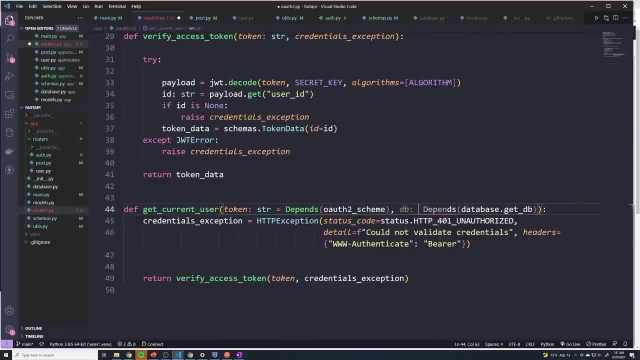 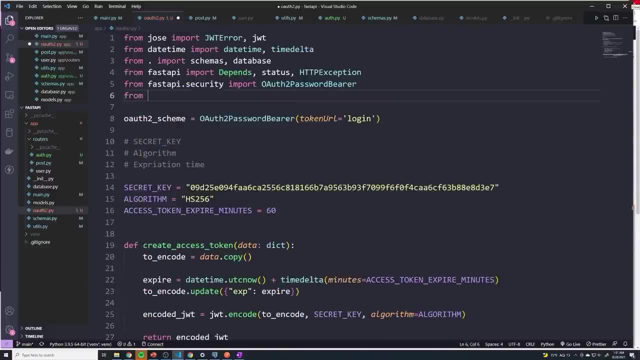 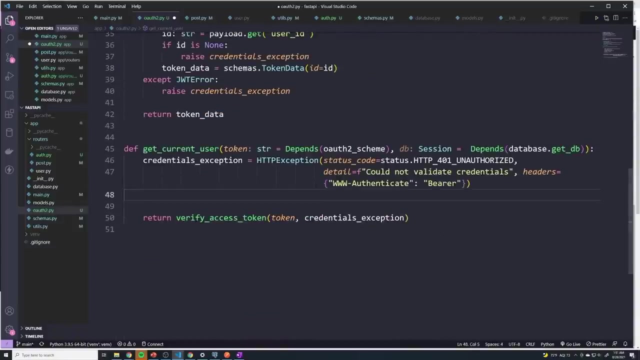 underscore DB And we'll say DB session equals. and then we have to import session from SQL alchemy, And so now we can make requests to a database, And what we're going to do here is, first of all, I'm no longer going to. 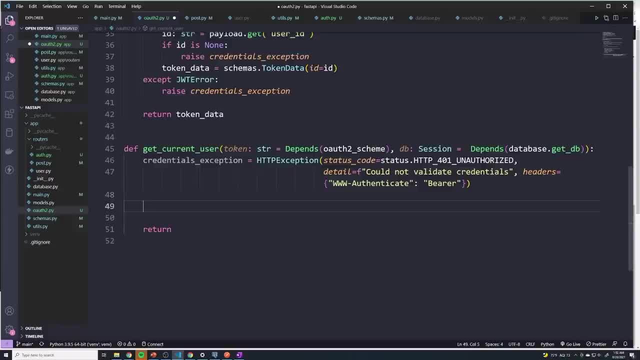 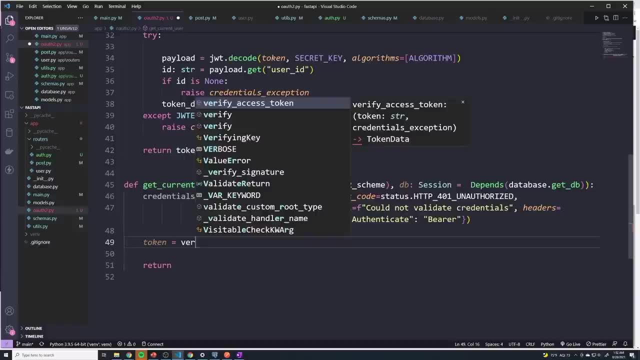 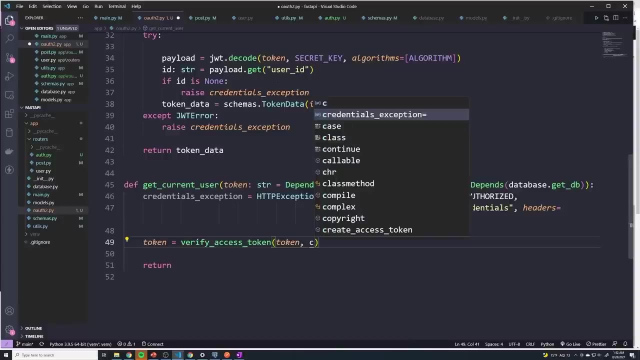 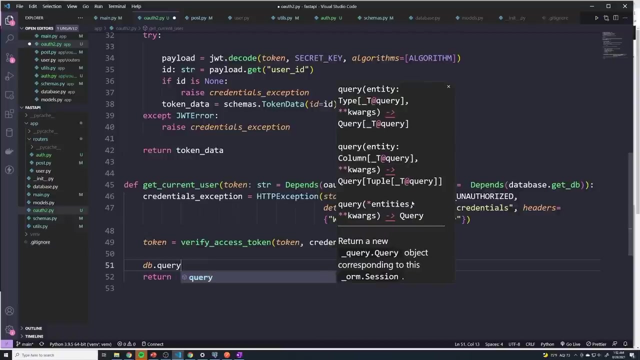 return that directly And I'm going to say token equals. and then we're going to call the this function right here, verify access, token Alright. and since we have access to the token, what we can do now is we can say DB dot query And then we have to import models, And I'm not sure if we've done that already. 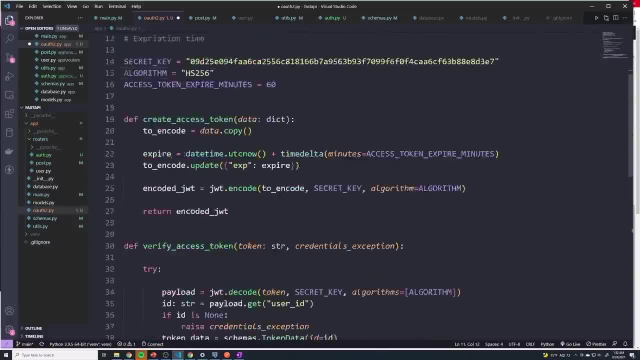 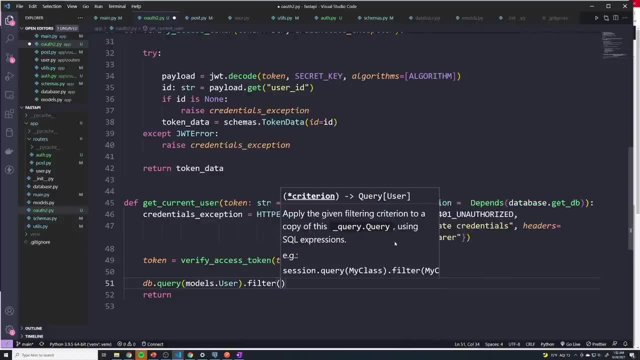 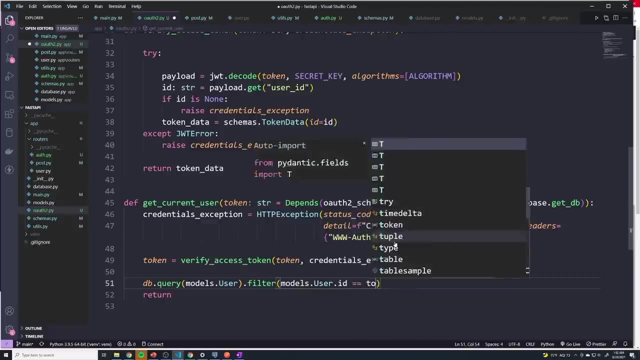 we haven't. So I'll import models. I'll say models dot- user, dot filter. and then we want to filter based off of the ID. So I'll say models dot- user dot. ID equals equals token, and then we just grab the ID field And then we're going to grab the first one And then 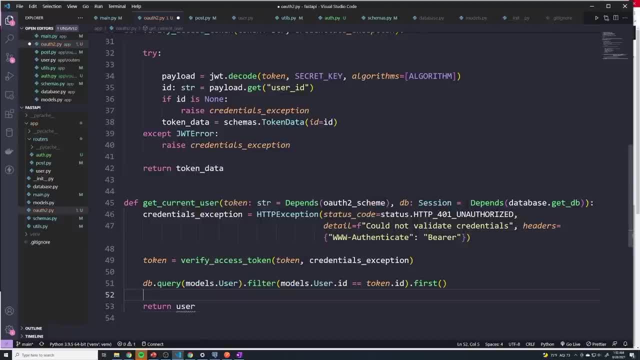 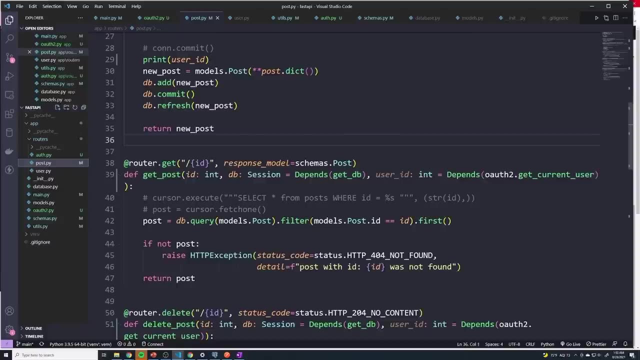 we can return the user which I forgot to save it. So user is going to be equal to the result of that And, if you want to, you can print user here. But I already know this is going to work, So we can just go and save this And then in our post app py right when we 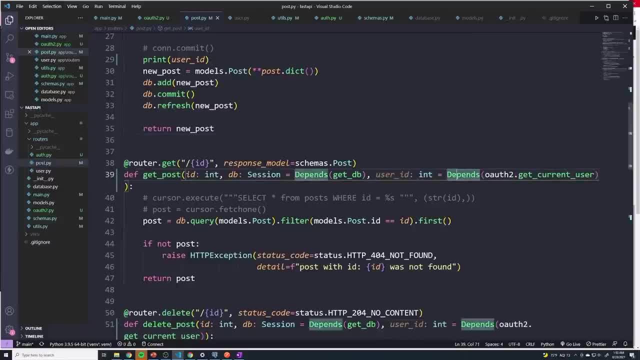 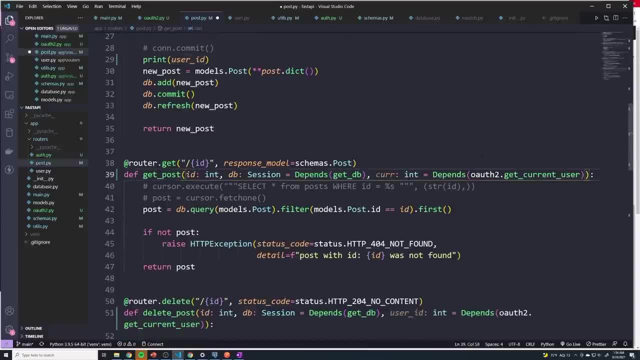 call this dependency right here. it's no longer returning the user ID, So I don't think it's it's a good practice to call this user ID anymore, because it represents a user. So I'm going to say I'm going to call this current underscore user. 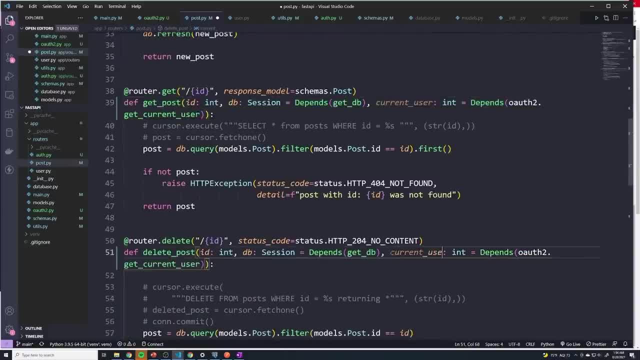 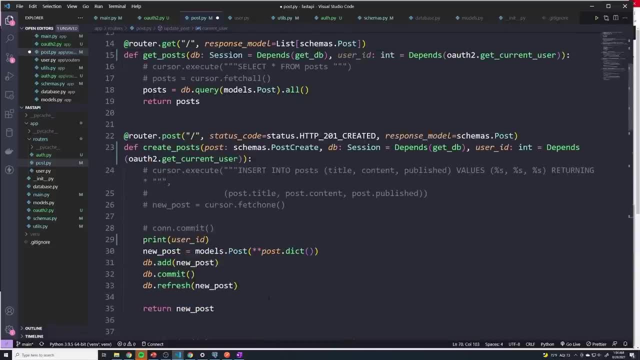 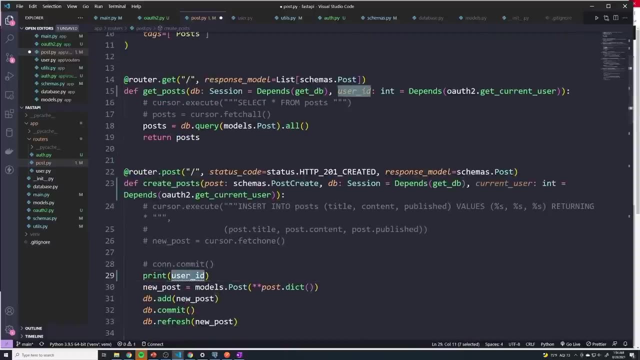 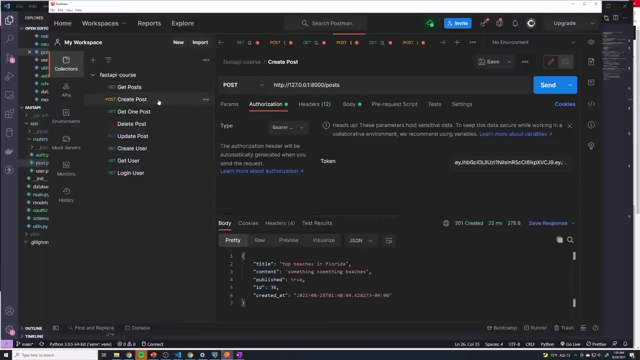 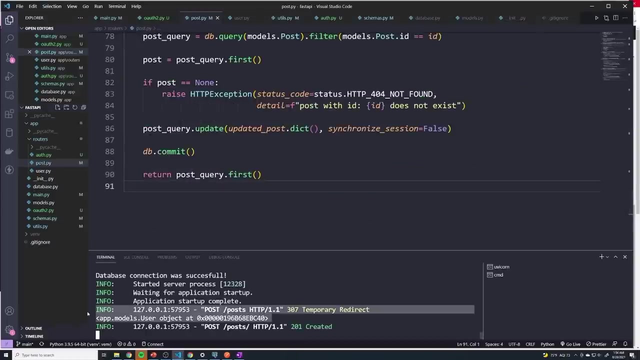 And we're going to rename this everywhere, All right. and then here within the function, I'm going to print out current underscore user. And so if I try to create a post now and then open up my console, you can see that it printed out the user object, which is not very helpful, But what? 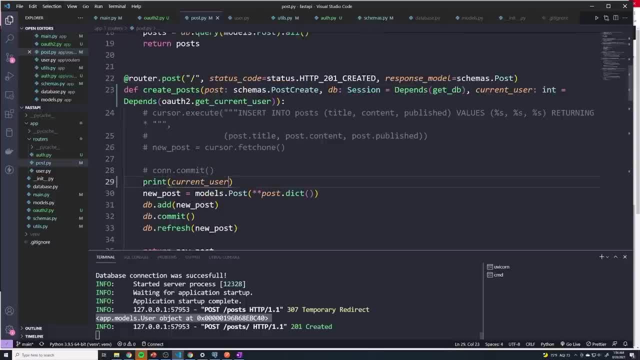 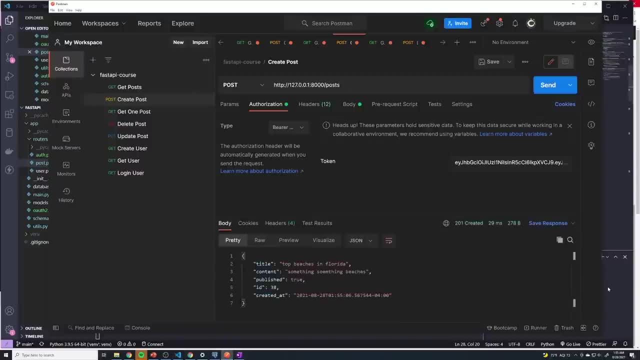 we can do real quick is, I'll just say, current dot user dot email. we can see the email of that user just to verify that we are actually getting the user And we can see that it does print out the email. So that's ultimately why this function exists, Because normally 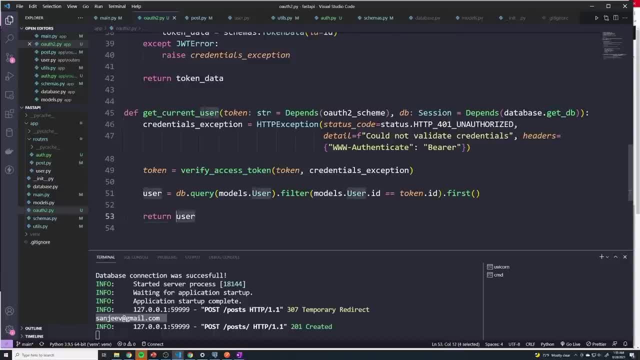 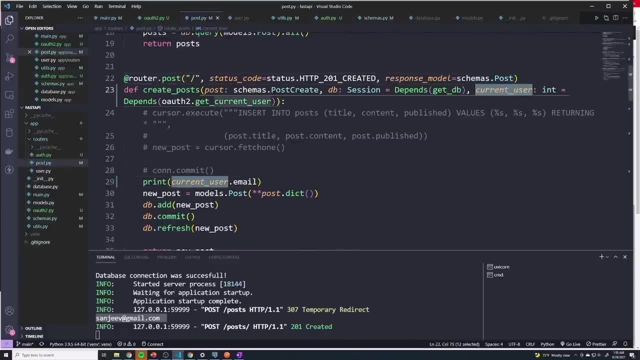 here. this is where you query your database to grab the user and then you return the user And then whatever you return here is ultimately what allows any of your other routes to get whatever you're returning. So since we're returning a user, we're going. 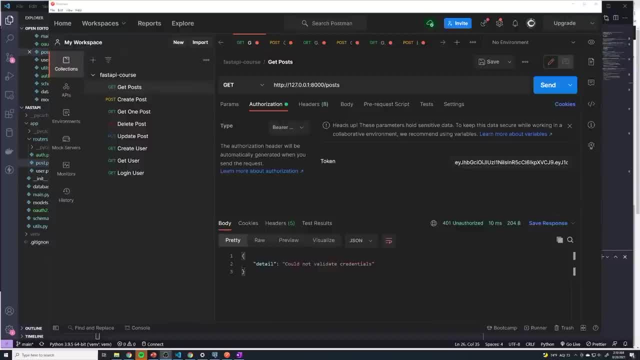 to store it as a variable called current user. In this video we're going to take a look at some of the more advanced features of postman, And we're going to start off by taking a look at environments. So select the environments tab And you'll see that postman just gives. 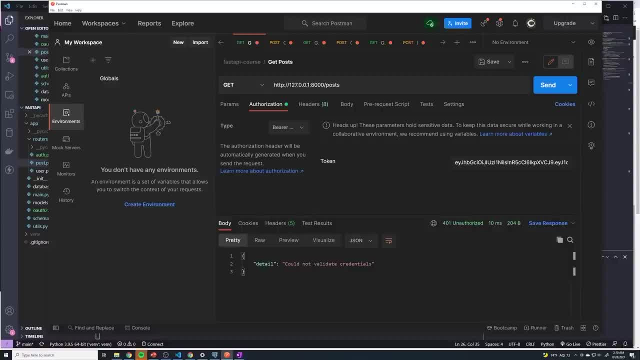 you a quick description of what an environment is. it says an environment is a set of variables that allow you to switch the context of your request, So we can set up some variables that change depending on what environment we work in. You're probably thinking: well, what exactly is the point of that? And let me give you. 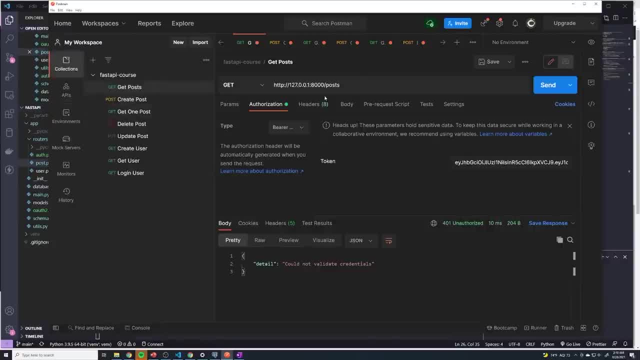 a great example. If you take a look at all of our requests, you can see that we have hard coded them to be 127.0.0.1, port 8000. And this is our development environment. Now, when we ultimately go to deploy our app, it's not going to be deployed on 127.0.0.1 to be. 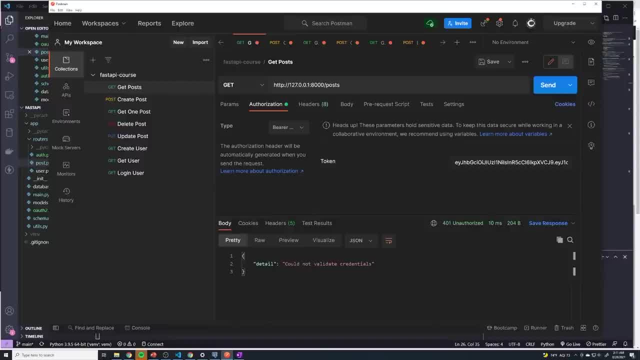 deployed on some server. it's going to have a public IP somewhere on the internet And so when we want to test out our production server or make some changes to our production server, make some test requests to it, we would have to change the. 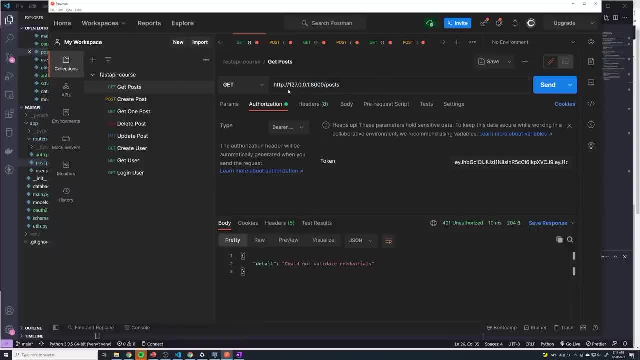 IP address, the port number as well, as we probably are going to be running HTTPS instead of HTTP. So all of our requests- we'd have to change all of them and then continuously flip back and forth every time we move from dev to prod and then from prod back to dev. 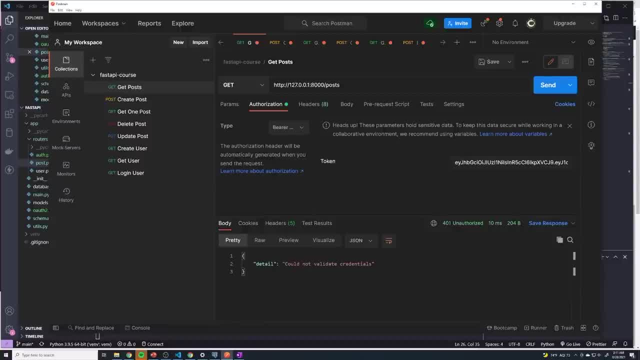 And so, instead of having to hard code these values, then change it constantly, we can actually create a variable that changes depending on what environment we use within postman. So let's go to environment And let's create an environment, And I'm going to call this 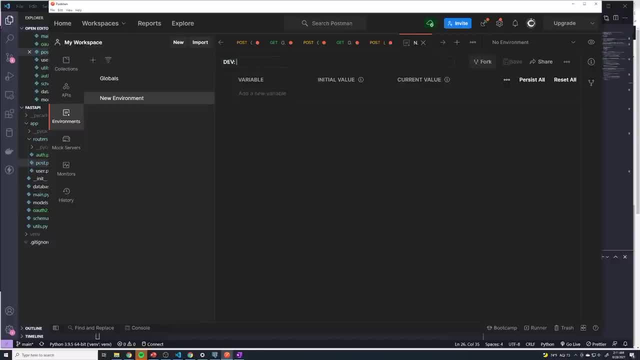 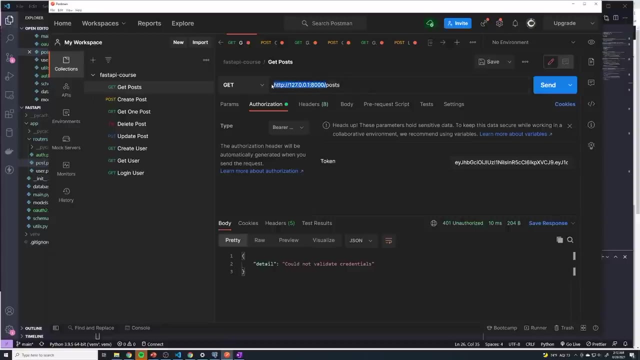 environment. we'll say this is dev, And then our project name, which is fast API. So this is our environment, And what we can do is we can define a variable and I'm going to call this one URL, And then here I'm going to actually just copy this URL. 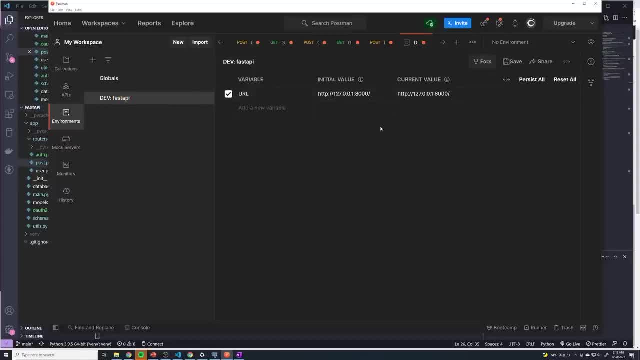 And then go to our environment again and I'm going to give it an initial value, Alright, and then our current value should update, and then we can just hit Save, Okay, and so we've set this variable to be this specific IP in our dev environment. So that's. 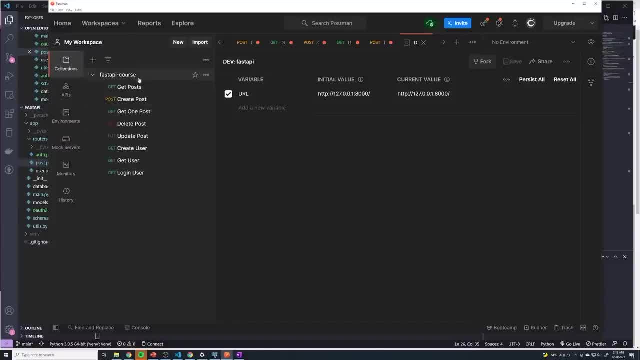 everything we need to do. So let's go back and just go ahead, and we're going to do the next step. So we're going to go ahead and add a variable to the environment, which is our environment, And so if we go back to collections and then go to our get posts first of all now, 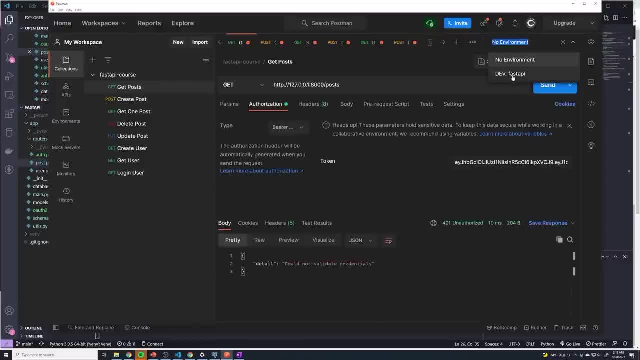 moving forward. you want to make sure that you're working in some kind of environment, So we'll select the environment we just created And then, instead of hard coding this value here, I'm going to change this And I'm going to just say to actually use a variable. you do curly, brace, curly. 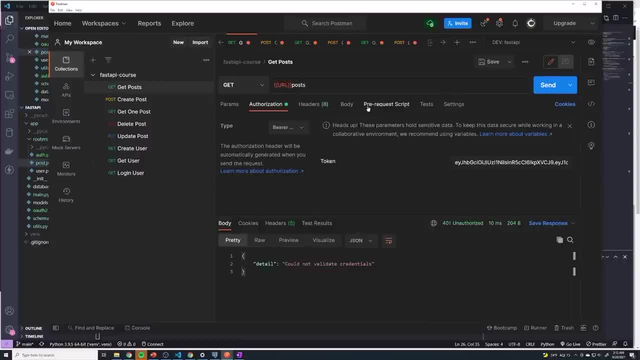 brace, the name of the variable, and then curly brace. curly brace, Okay, and it should be orange instead of red. if you get a red, it's going to meet in that it wasn't able to resolve something and there's some issues. So just double check what you did. Orange is good And then, if you, 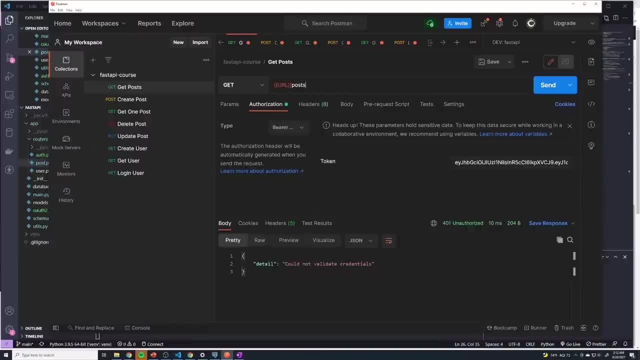 see this result when you have over hover over it. that means that everything's working, And so, just to quickly test this, you can see that it says could not validate credentials. that's perfectly fine. I didn't set up the access token or anything, But this does confirm that we're able to. 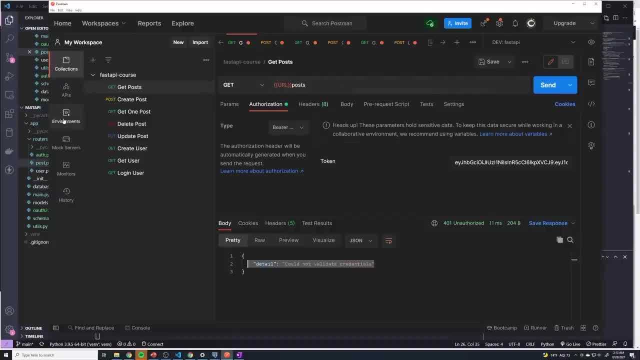 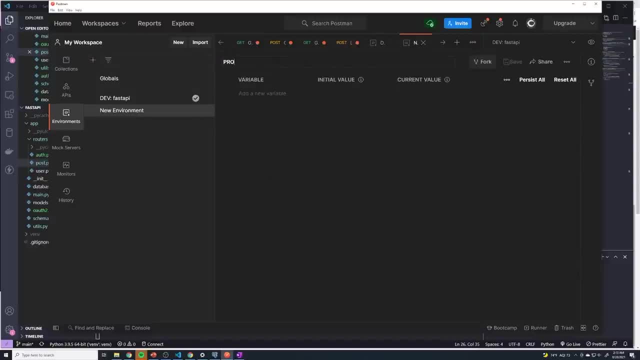 resolve that variable And so that way you know, if I go and then create a new environment and I'll just add here and then we'll say this is prod Fast API, We can then give a different URL for the production environment. So this could be like: 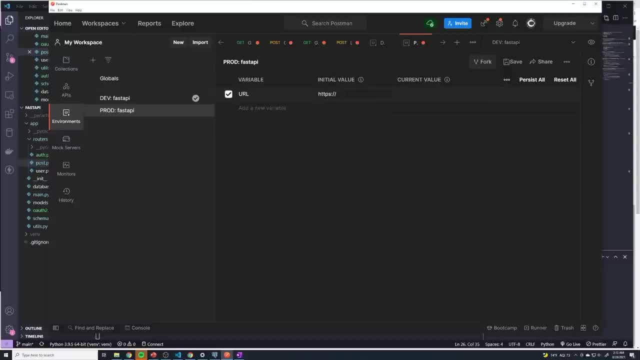 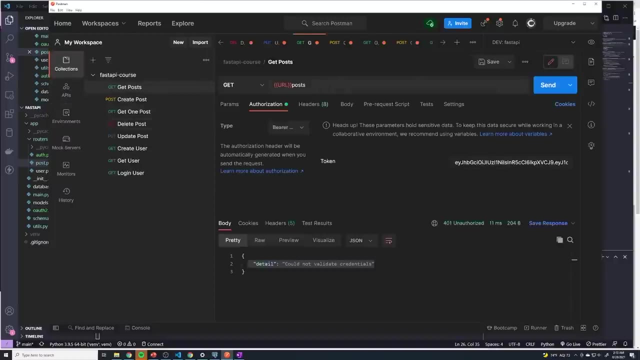 you know HTTPS, colon slash, slash, I don't know. you know some domain name that you buy. I'll call this Sanjeev, dot x, y, z, slash, And then I can save this, And so that way, if you ever are testing your development environment, 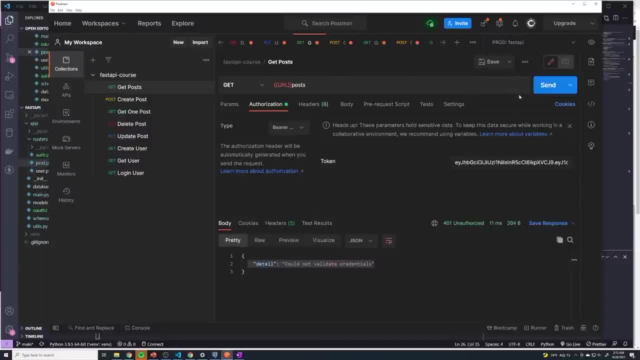 you just go to dev And then, when you want to quickly switch to your production, you just change that and then the URL will automatically update. So you don't have to change anything yourself, And it's super handy to set this up, And we're just going to do this. 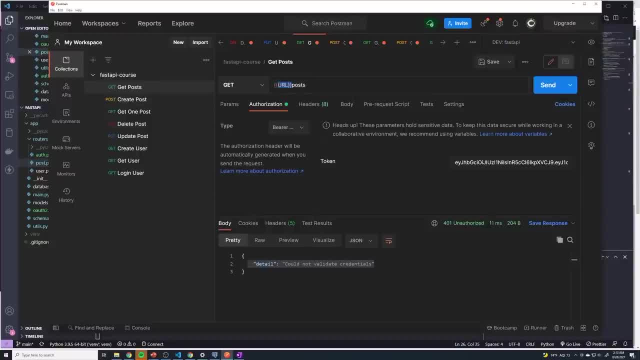 for all of our requests moving forward. So I'm just going to copy this And we're gonna do this for all of them. Okay, and if you go ahead and test this yourself, you should ultimately not run into any issues going to bore you through. you know, individually testing these, you can do this yourself. 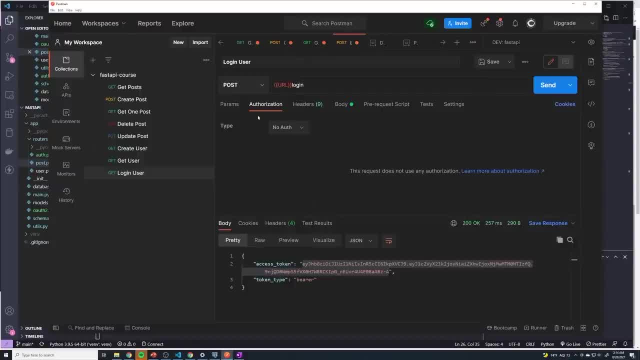 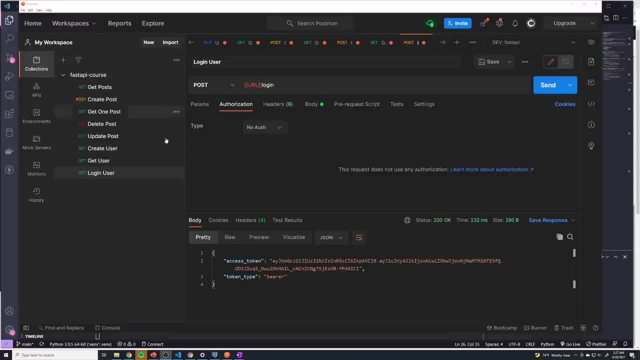 And, if you know, if you run into errors, it's just you probably paste it in something wrong. Now that we've set up authentication on our API, testing our API has gotten a little bit more challenging, And that's because I can no longer just go to create posts. 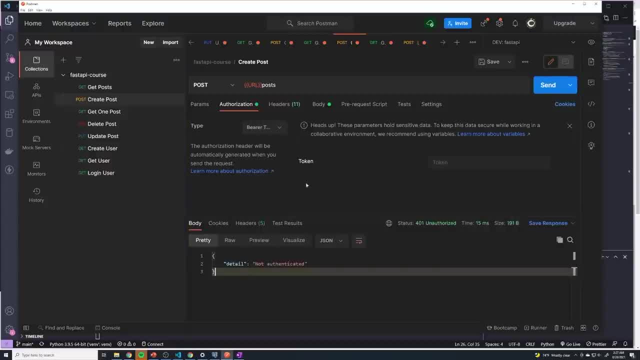 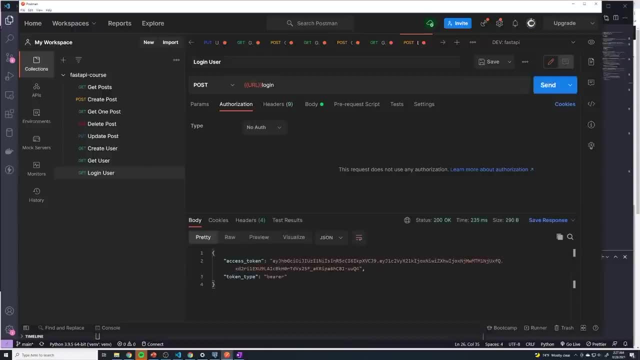 and then just hit send. because I have to be authenticated first to be able to actually create a post. And so what I have to do in postman is I have to hit send, I have to log in and then get the access token, I have to copy the access token. 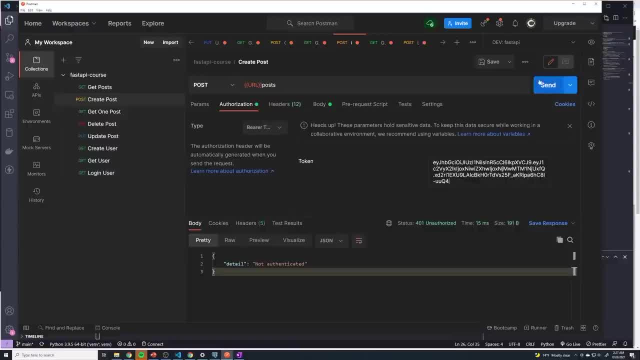 And then go to the specific endpoint I want to test and then I want to paste that in there and then hit send And then I can finally create post. And this is a little cumbersome and tiring And it gets really hard if you have a short expiration time on your token. Imagine if you 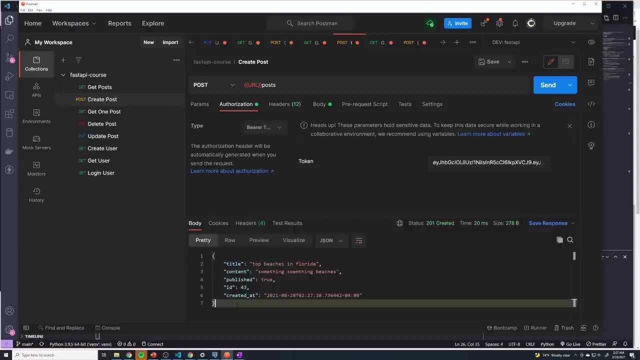 had an expiration time of five minutes, then every five minutes you'd have to repeat this process, But luckily postman has a way to actually do this through an automated fashion. I, we're all developers, we all want to do things automated. So let's take a look at how we can do this, And I had 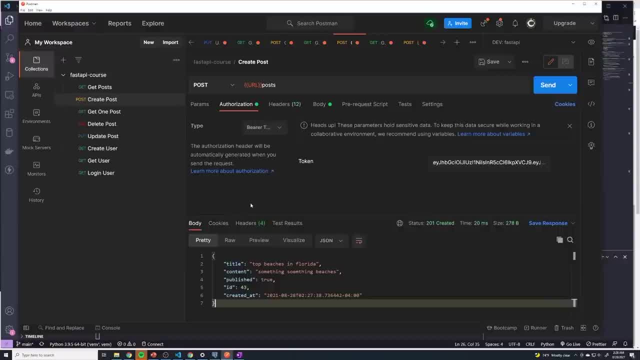 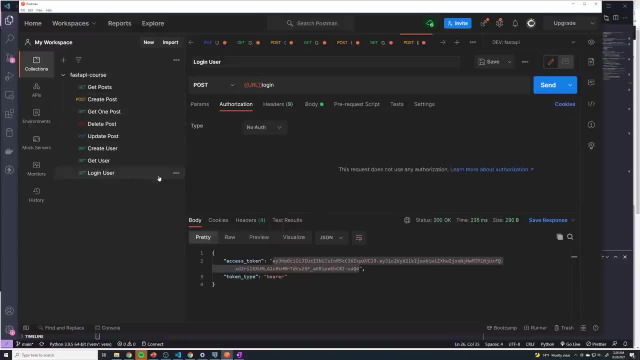 to make sure that you can see this. So let's take a look at how we can do this. And I had to make sure that you guys understood environments and variables beforehand, because this, the method that we use, actually makes use of environment variables. So let's go to the login user endpoint. 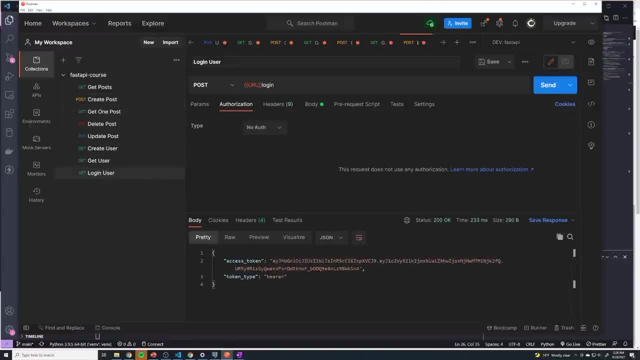 And we're going to hit send and get a new access token. And so we've got this access token And what I want to do is, through code, I want postman to automatically set an environment variable. So how do we do that? Well, let's go to tests And here we can put in whatever code we want. 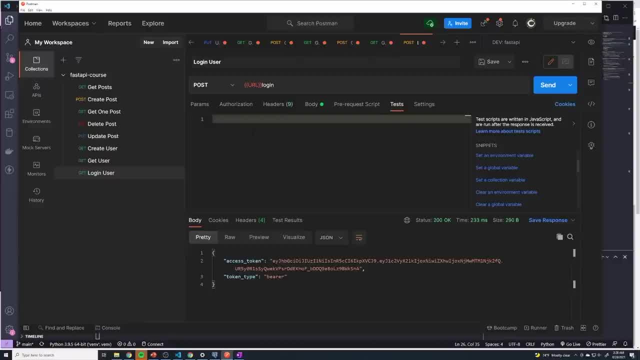 And so we can read the documentation on how to do this, But the ultimate goal is to set an environment variable through code. So how do we do that? Well, there's a little snippet here that kind of gives you examples, And what we want to do is we want to set an environment. 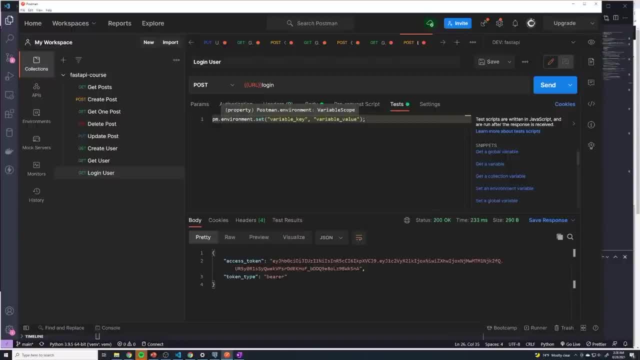 variable. And so to set an environment variable, you just do environment dot set, provide the key and then the variable name, And so, just like we did with environments, right, if you go into your environment, you've got the URL, which is the key, and then the value, And so we're just. 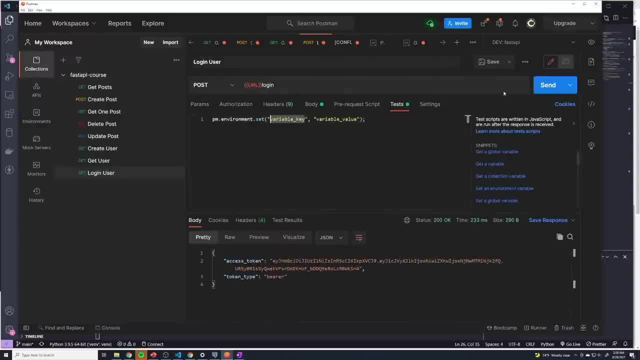 going to do the same thing, but just through code. So here I'm going to set the key to be JWT And I'm going to set the value to be this access token. So how do we actually retrieve the access token from the response of the request? Well, we can do pm dot response that grabs the. 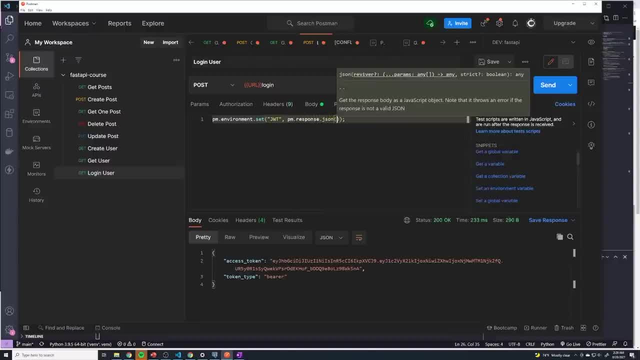 response object, then we'll convert it to JSON And then we need to get the token, and the token sits on a property called access underscore token. So whatever this field is called, this is what you're going to pass in. we'll say: dot access underscore token. Alright, and so now. 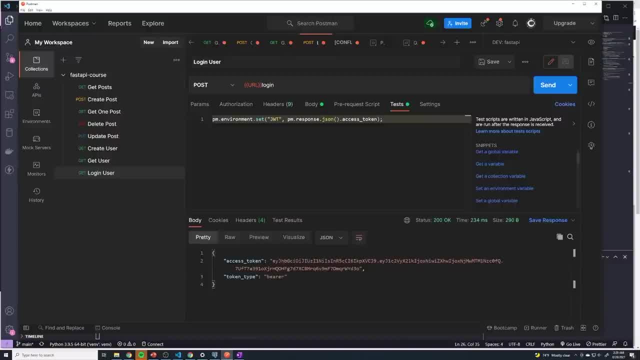 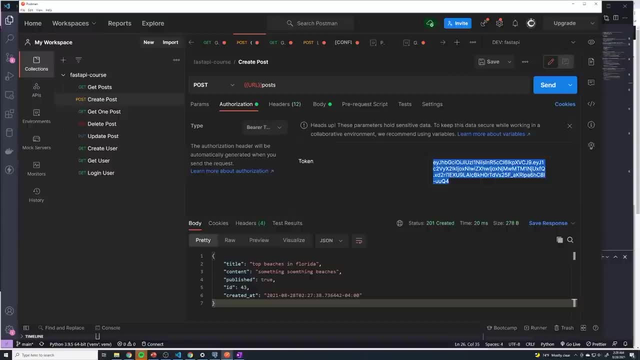 we're going to do this again. we'll get the token, the code should have run and it should have set a variable called access token. And so now, under create post, instead of hard coding this, what I can do is I can actually just reference the JWT variable, And so I set minus capitals. there looks. 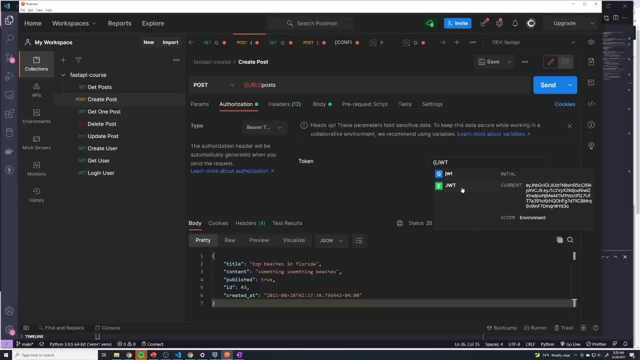 like there's one from a previous project maybe, But we want this one right here. And if you want to just double check, you can see that this ends in w y d three. Oh, and if you want to go back into a login user, you can go back into the login user and you can see that this ends in w y d three. 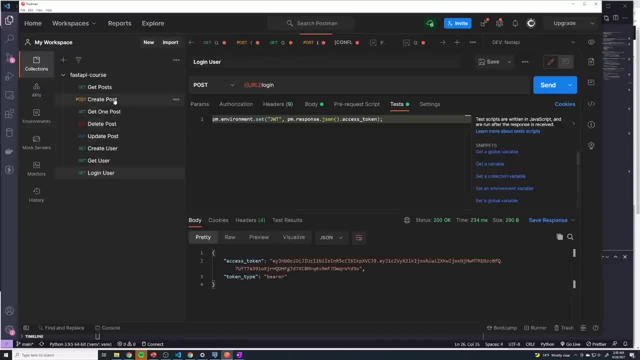 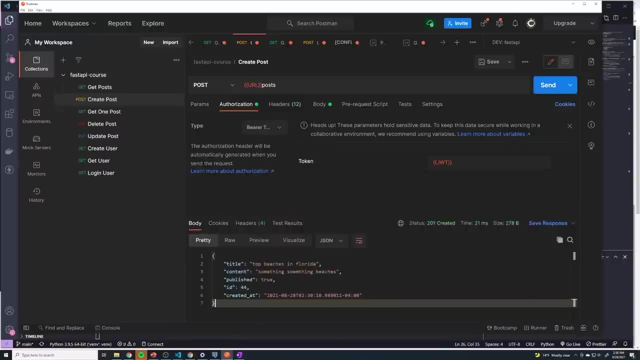 Oh, so it looks like it did set that and update it accordingly, And we'll set that in there, And so now, if we send, you can see that it we can now create posts, And so anytime you log in a user. 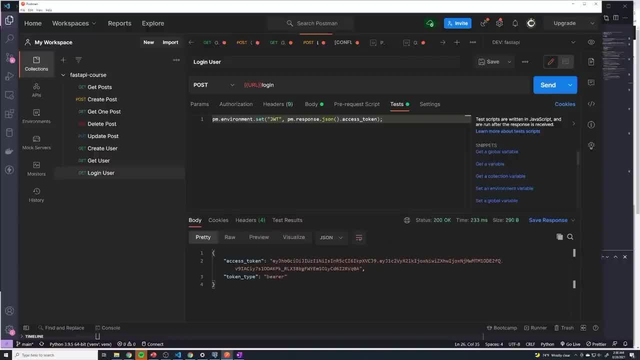 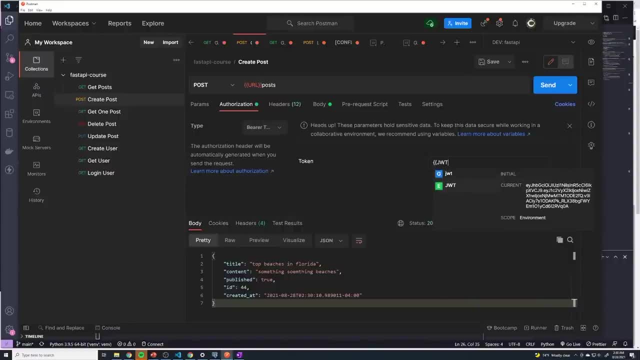 it's going to update that token And we can verify this. if you take it, the last three letters, q zero a is the new token And then I'm going to just remove that So we can see the value And we can see that q zero a is the last three letters as well. So this update is going to update that token. 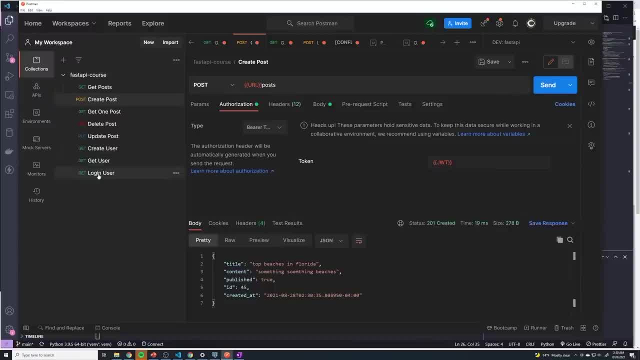 And it updates it dynamically, so that all you have to do is now just hit login user And then you can start testing all of your other endpoints. And we're going to update all of the other endpoints as well, So forget posts. I'm going to put that in there as well. And then for getting. 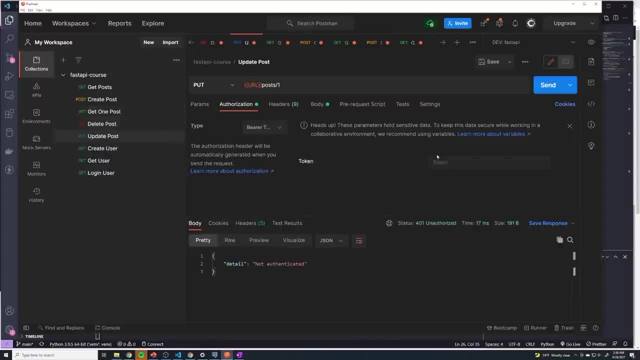 an individual post, deleting a post, updating a post. we don't need it for create user. we might want to do a forget user if we set up authentication for get user, but we haven't done that yet, So we'll hold off on doing that for now. 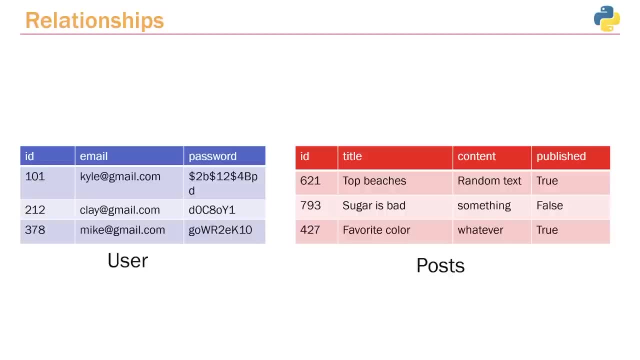 Now, currently, our application doesn't work like a traditional application would, And the reason I say that is, you know, if you take a look at how everything's been set up, not just in our API but in our database. we've got two tables: a user table and a post table. 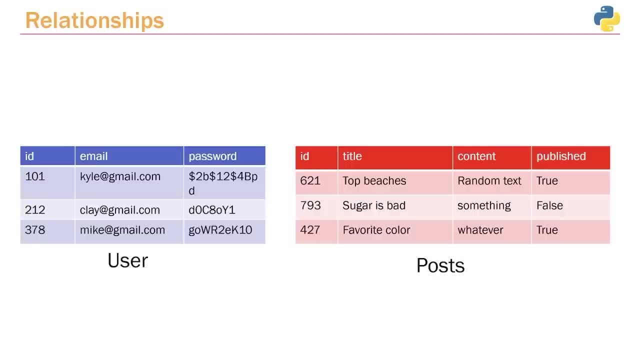 So we can create, modify, delete users however we want. we can log in And then we can create, modify and delete as many posts as we want. Right, And you probably think: well, that sounds perfectly fine. Yes, However, think about any other application. 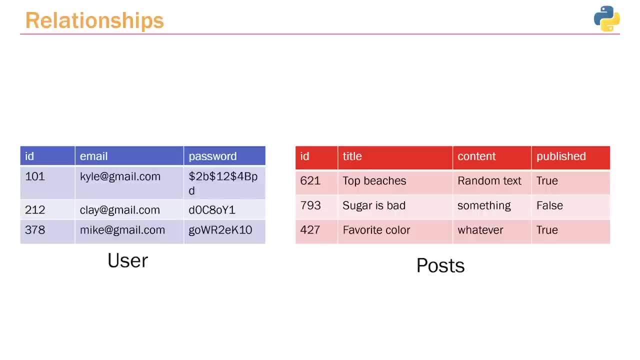 about any social media type application. when someone creates a post and you see that post on your feed, what are you going to see next to the post? you're going to see the user that created it, right? So every post is ultimately associated with the user account that created that post. 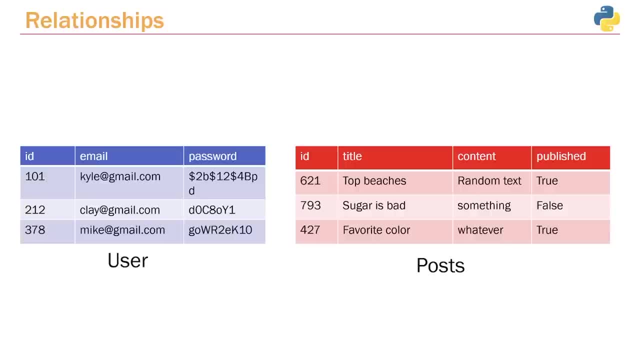 But we have no way to actually do that in our application at the moment because there's nothing that ties a post to the user that created it. I take a look at all of the columns in our database. we've got an ID, a title, content published technically. there's a created. 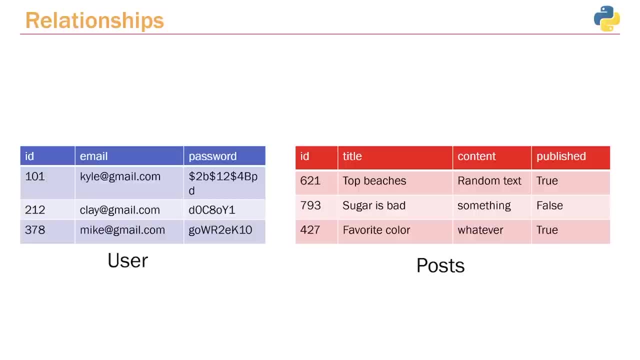 that column that I didn't draw in this diagram, but that's okay. So how do we know what post was created by what user? And this is where relational databases really start to shine, Because the main idea behind a relational database is that you set up these relationships between tables. So we need 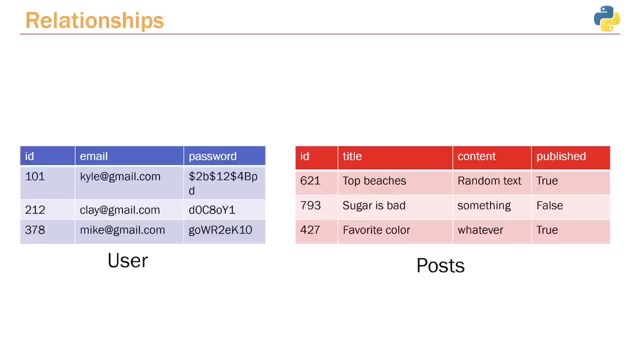 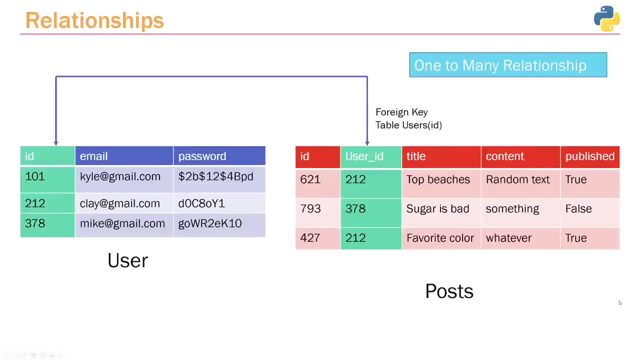 to set up some kind of special relationship between the users table and the post table that will allow us to associate a post with a specific user that created that post. So let's do a look at how we can do that within Postgres or any SQL based database And the way we do that is. 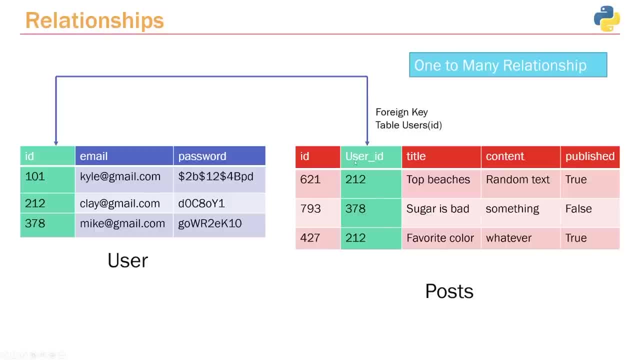 we actually create an extra column in our post table. So we've got a column. you can call it whatever you want, But I'm going to call it user ID And I'll explain why. And what we're going to do is we're going to set up a special foreign key, And a foreign key is a how we tell SQL that this 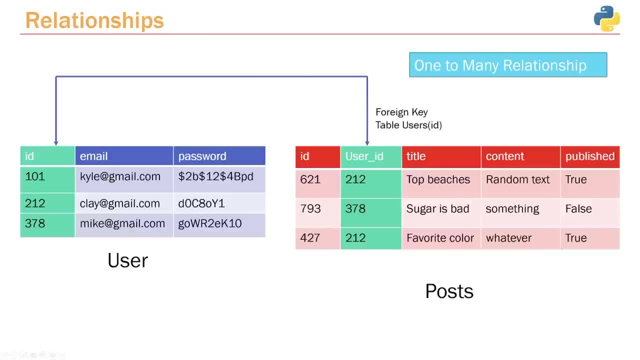 column here is connected to another table, And what we do is we specify two things. We specify the table that it should be connected to. So here I'm saying, hey, this should connect to the user's table. And then we specify what specific column it should use from that table. And here we're. 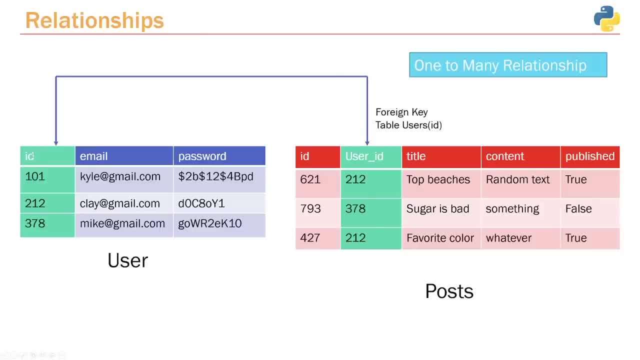 saying the ID call, because this connection is connected to the ID column of the users table, And so that's what we set the foreign key on, And all this is does is? this is really such a simple concept. Whatever user creates this post, we just embed the ID of that specific user. 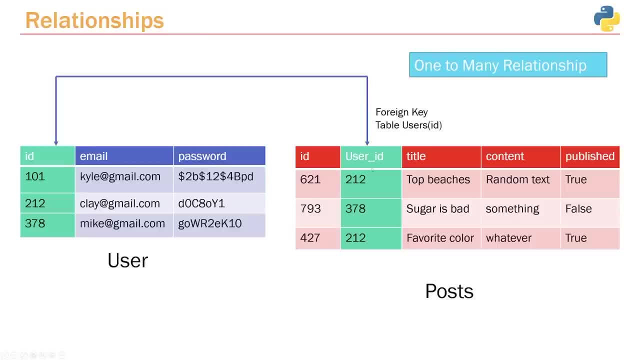 So, for the post with the idea six 21,, the user that created this has an idea of of 212. So if we take a look at what user has an ID of 212, we go here and we can see that clay at gmailcom created this post, And so that's all we have to do to set up a relationship between. 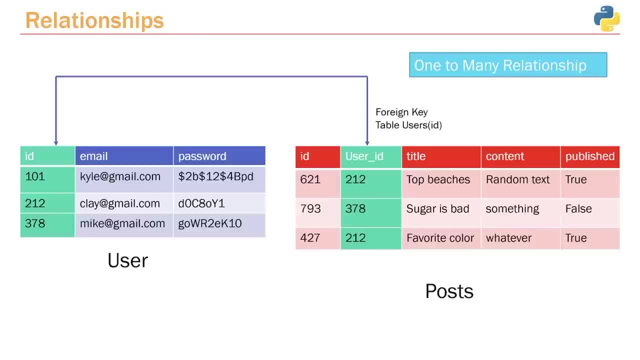 these two tables. And so now, moving forward, any post we create, we'll easily be able to tell what user created it, because we're going to embed the ID of that user into this column called user underscore ID. And if you take a look at the second one as an example, we can see that this: 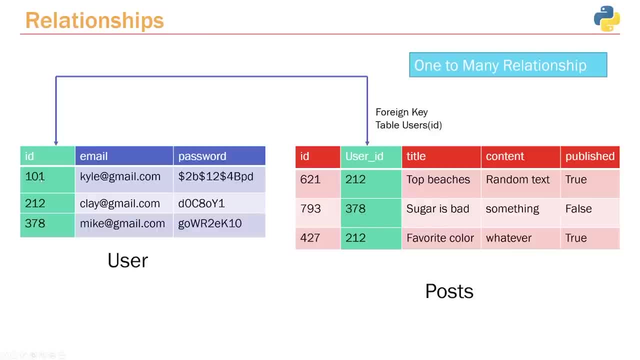 was created by a user with an ID of 378.. So we go into the user table and we can see that this user is Mike at gmailcom, And it really is as simple as that. And this is what's referred to as a one to many relationship within SQL or any relational database And the reason why they call 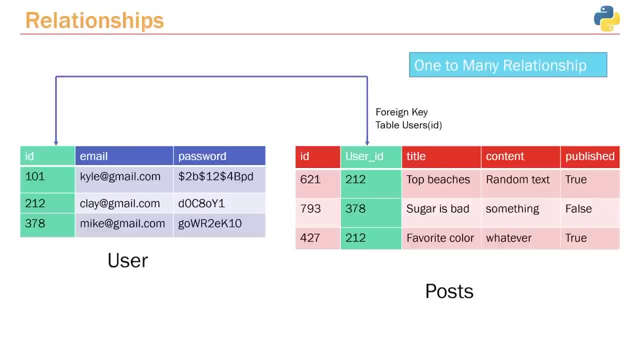 it. that is because one user can create as many posts as they want. However, a post can only be associated with one user. two users can't create a post, And so that's why this is referred to as a one to many relationship. one user can create many. 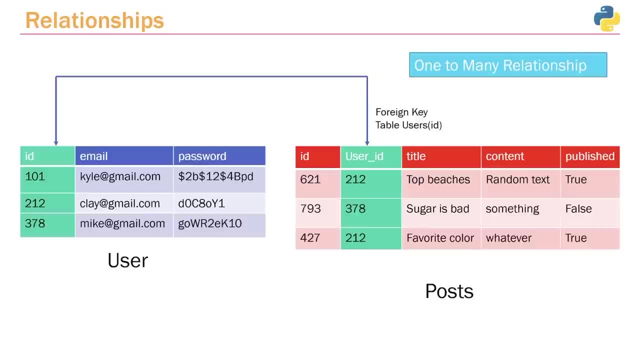 posts And that's all we have to do. It is actually that simple. we just create another column And then we have to specify this special foreign key constraint where we just tell SQL: hey, what table do we look for And what column And keep in mind? in this case I'm using the ID of 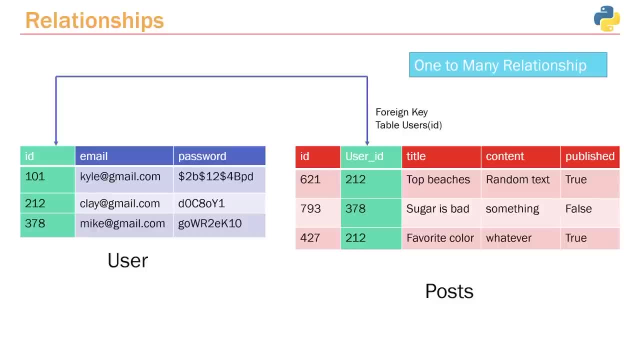 the user's table. But when you get a little bit more advanced with SQL and setting up relational databases, you'll find that it sometimes you don't have to always set up a relational database to always point to the ID of another table. there's- there's going to be- a lot of instances. 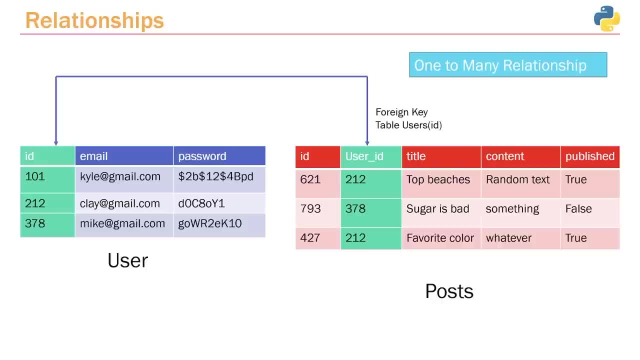 where you set up foreign keys to other columns that aren't necessarily the ID column. depending on how your relationships are set up and how your application should work, That is a perfectly acceptable thing. There's no specific restriction saying that it has to point to the ID column of. 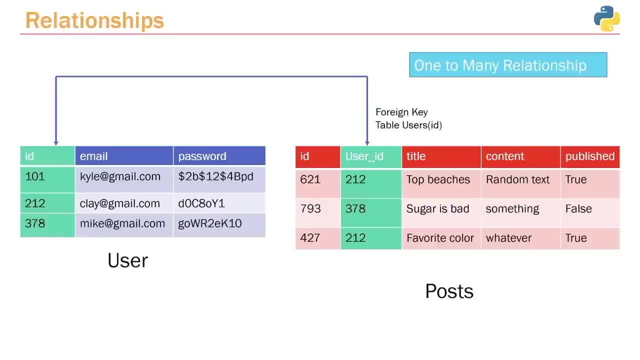 another table And so I think that's enough theory behind foreign keys and relationships. So we're going to connect to our Postgres database in the next section And we'll start creating that extra column adding the foreign keys, and then we'll start creating that extra column And then we'll 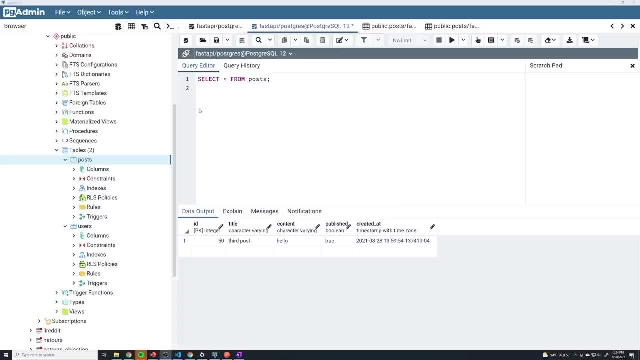 start learning about how to actually work with these relationships. Okay, go ahead and open up PG admin And before we get started, I'm going to do something a little unusual: I'm going to delete everything from our post table. Now, when it comes to creating an extra column and creating a foreign. 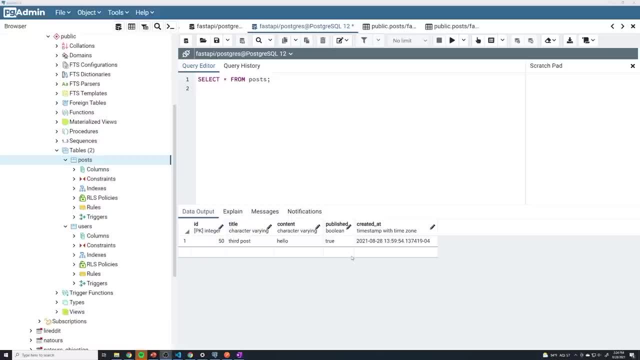 key. that's not a requirement, you know you don't need to do that in a production database. I'm just going to delete everything, just to keep, just to make things a little bit more simple moving forward, Because if we don't delete anything when you start to add columns, that 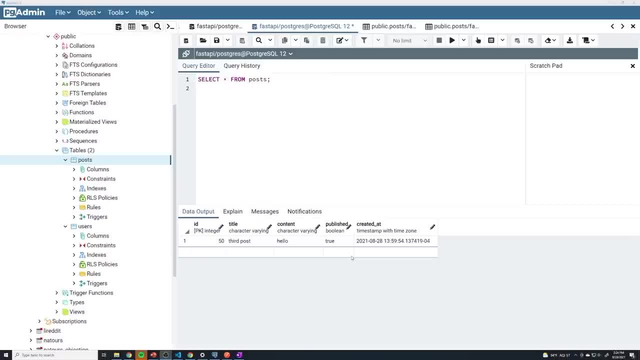 especially have a not null constraint. we have to do a little magic to kind of get that to work, And I want to keep things as simple as possible. So what we're going to do is we're just going to delete everything from the post table, just to make things as simple as. 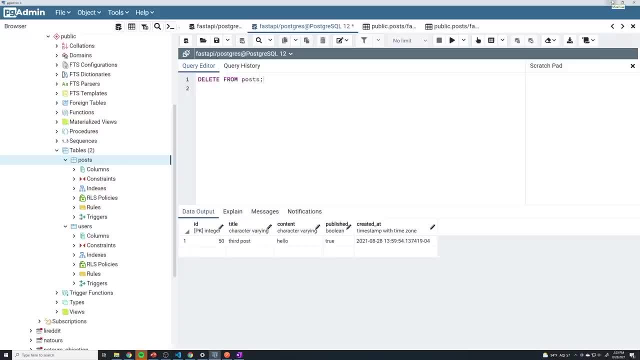 possible. So we can just say delete from posts And that should delete everything and everything's gone And we should be pretty much good to go to actually start setting up our foreign key. So right click on your post table and then click on properties And the great part about these foreign 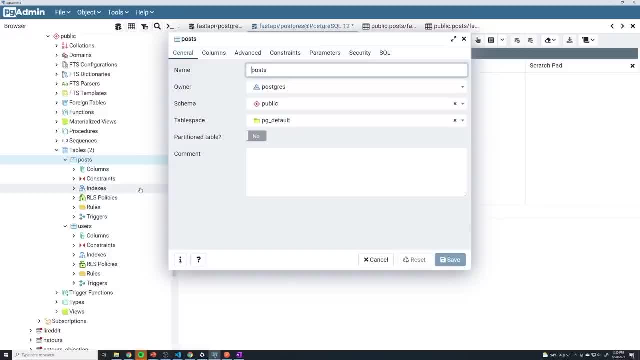 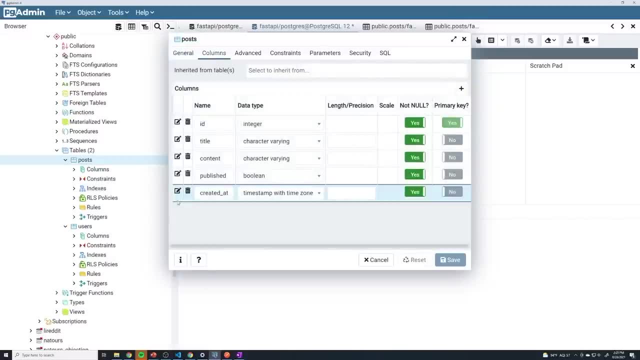 keys is that you know we just have to do this on the post table because it's a one to many relationship. there is nothing in the users table that we have to do. So what we're going to do is we're going to go to column And then we're going to add a new column. 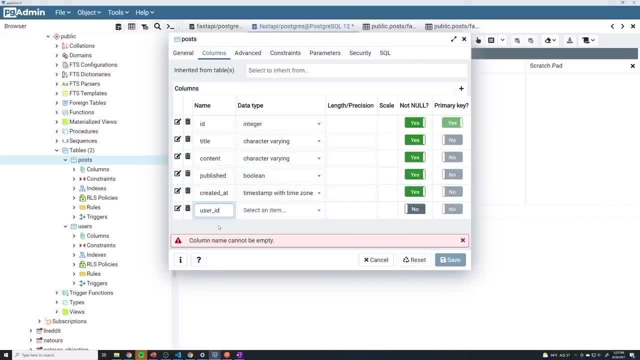 And I'm going to call this user underscore ID And you can once again name this anything you want. the actual name doesn't have to make sense, But you know, I think naming it user underscore ID makes sense, because this is a column that's going to represent the ID of the user that created our 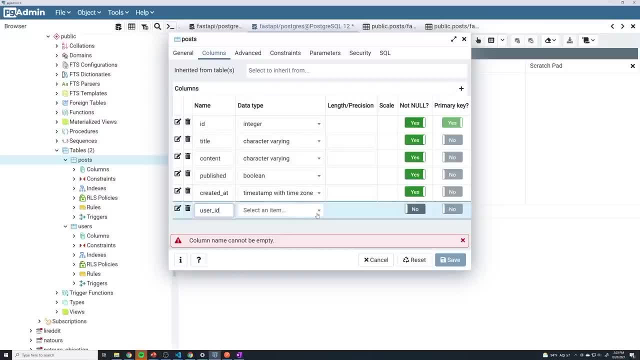 post the data type. Now, this is important because the data type of this column needs to match whatever the data type is of the ID column from the users table. So we always set the ID up to be integer, so you want to match this. However, keep in mind that sometimes, when you're working with data, 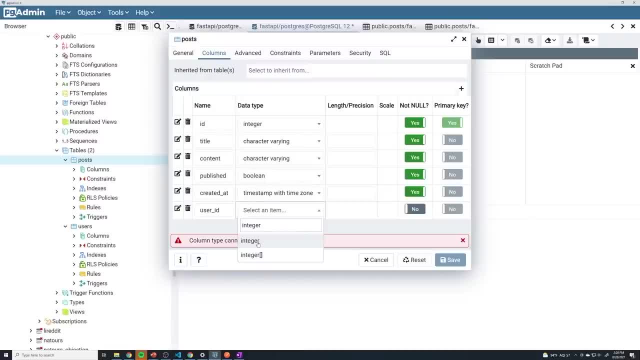 spaces. it might be some other data type, right? If you use big int, you definitely want to make sure that this is also a big int. if you use a small int, make sure there's a small int. If you use UUIDs, make sure that this is a UUID as well. you just want to match up with whatever that. 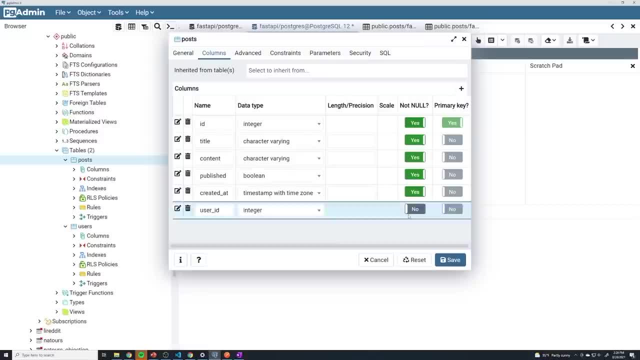 column is in that respective table. Now we have the options to set this as not null, So right now we can create a post With a null user, which means there's no user that created this post. And if, and to figure out if you. 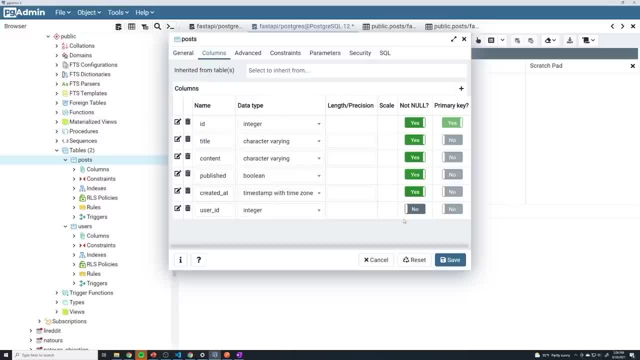 should set this to be not knowledge. it depends on how you want to set up your application. Should the database allow you to have a post without a user? It's up to you to decide. I'm going to say no for now. I'm gonna say not, not because I don't want to be able to create a post without a user. 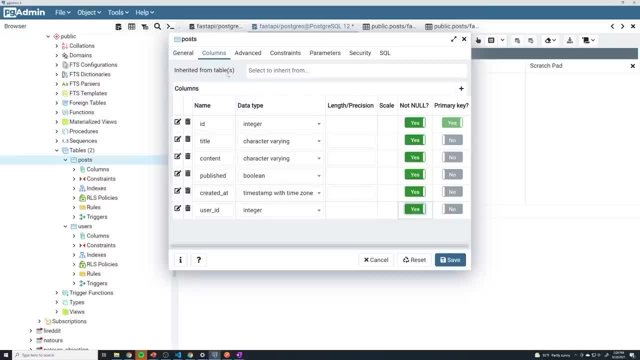 It doesn't make sense. And then after that what we can do is we have to set up our foreign key constraint. So let's say we want to create a post without a user And then after that what we can do is we can set up our foreign key constraint. So let's go to constraints, And then we want to go. 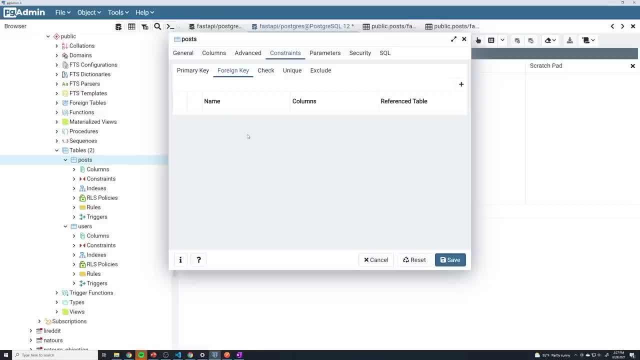 under foreign key. So this is where we set up that magical connection between the two tables. hit the plus sign and then give this foreign key a name. the name of the foreign key doesn't matter, Right? it doesn't impact the functionality of the thing. This is more just for you as a user to be able to. 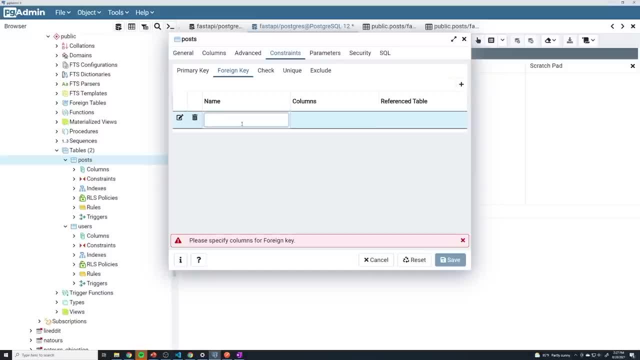 read it a little bit more clearly when you see it on the CLI. But there's a standard convention that we like to use when it comes to naming our foreign keys. What we like to do is we like to take the table that we're working on, so it's going to be posts, And then we do underscore, then the table. 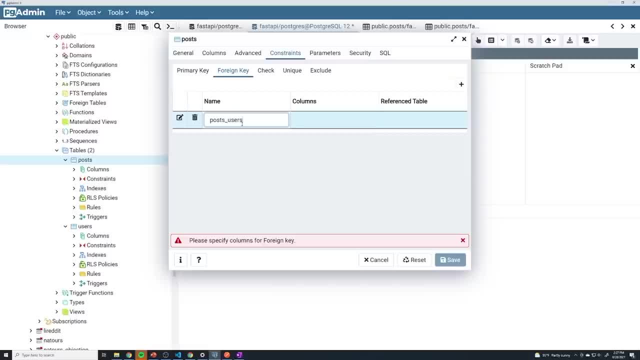 that we want to set a foreign key to, so it's going to be users, And then we just do underscore F key. Once again, this is just nothing more than a name to describe the foreign key. it's not actually doing anything at the moment. To actually set up the logic of the foreign key, we have to open this. 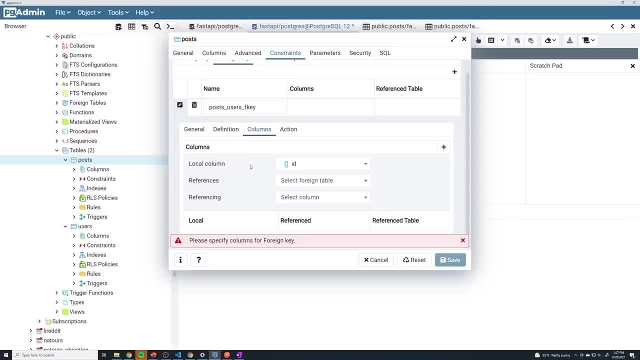 up And we have to go into columns, And so this is how we actually set up the relationship. So here we're going to be using what is the name of the local column, the column in our posts data table, what we created, our brand new user underscore ID. then it's going to reference what table. Well, 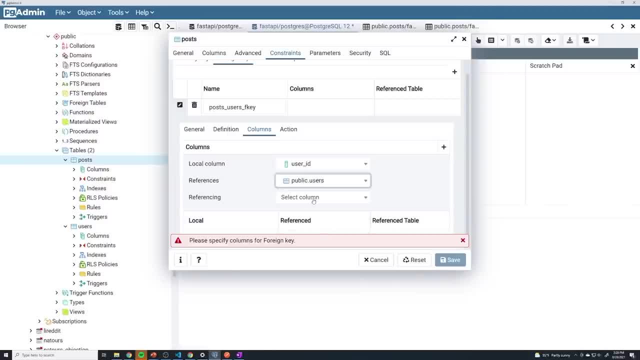 we know it's going to reference the users table, So we select the users table And then what column from the users table is it going to reference? Well, it's going to reference the ID column of the user table, And at that point you just hit plus, it gets added up here. And before we move on, 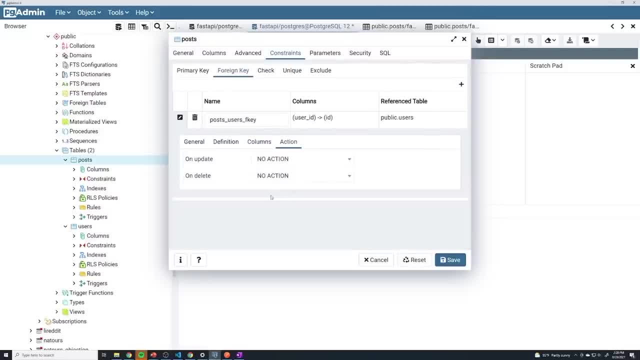 there's one last thing I want to cover, Almost done. we have to go under actions And, because we're setting this relationship up between two different tables, we have to figure out. you know what happens when a user gets deleted. right, Because right now a post is going to have the ID of the user that created it. what if we? 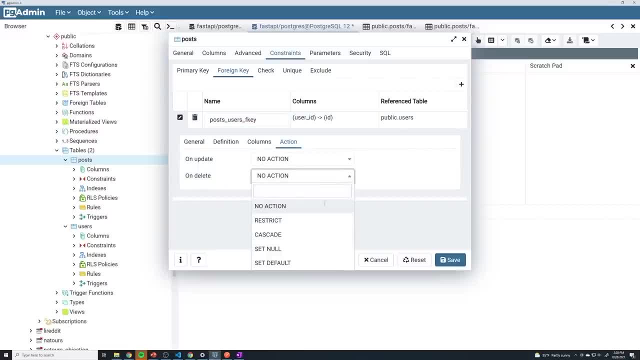 delete that user. What do we do? So if you go to the on delete section, we have a couple of different options. One of the more common ones is cascade, And so what cascade does is if I, let's say, if I have a couple posts that were created by a user. 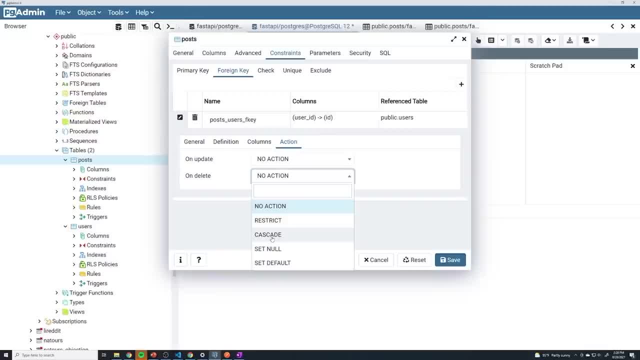 with an ID of seven. if I delete that user, then Postgres will automatically go into my post table and delete any posts that were created by that user, And so that's one option. That's what I'm going to use. However, we have other options as well. We can set it to the default value of a. 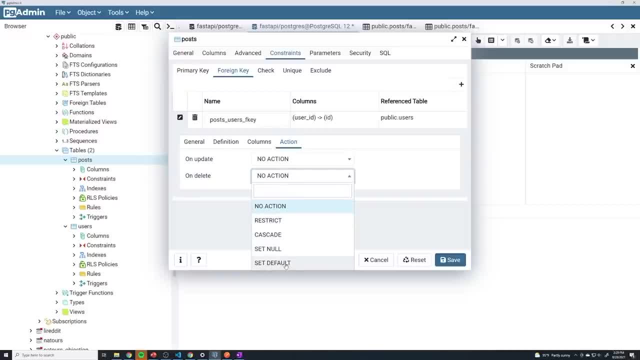 column. So if we give the column a default value- maybe we create like a, like a random ID of zero or something- then it's going to assign all of those posts that were created by the deleted user to zero. we can set it to null. So if we delete that user, we can set it to null. So if we give the 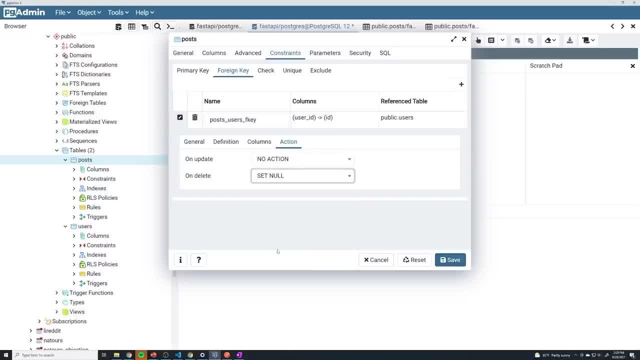 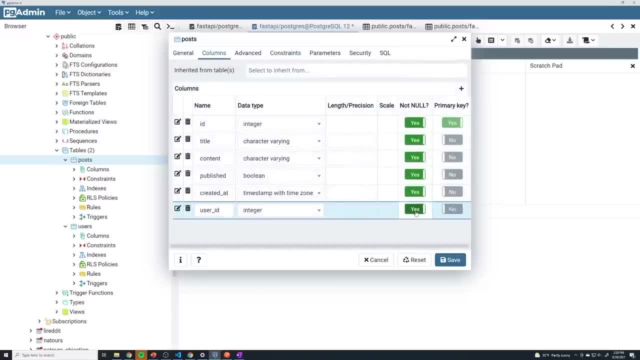 set null, then it's just going to set the user ID column to null if that user gets deleted. Keep in mind, if you want to be able to use set null, then you have to go back to columns and make sure this is not set to allow you to set it to null. So we'd have to set it to no or then it would throw an. 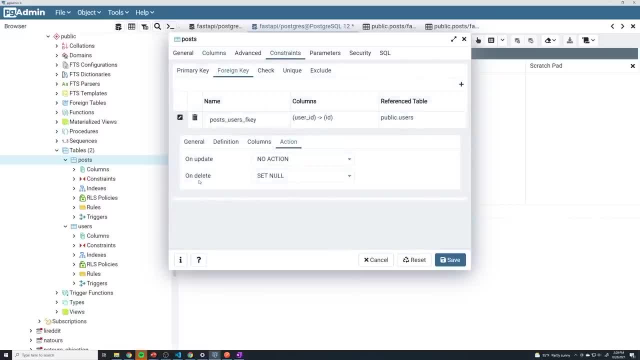 error when you try to delete someone, And then there's a few other options, But we're going to stick to cascade And then keep in mind you can do the same thing with on update. So what actions do you want to perform when you update a specific user in that case? but we'll leave it at that. 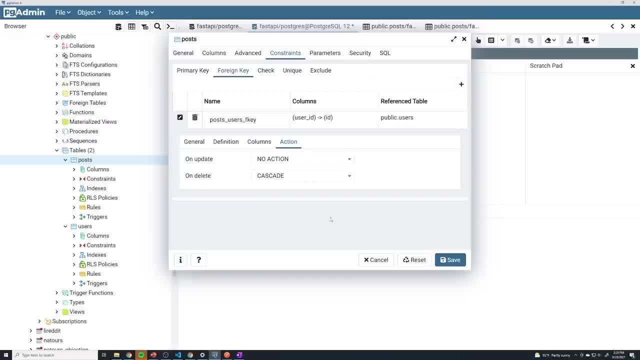 No action for now. I just mainly care about the on delete At this point. that's all you have to do for foreign keys. you just specify the column of the other table it should point to and you're good to go. We'll hit save And then we're going to go under posts. Well, actually, before we do, 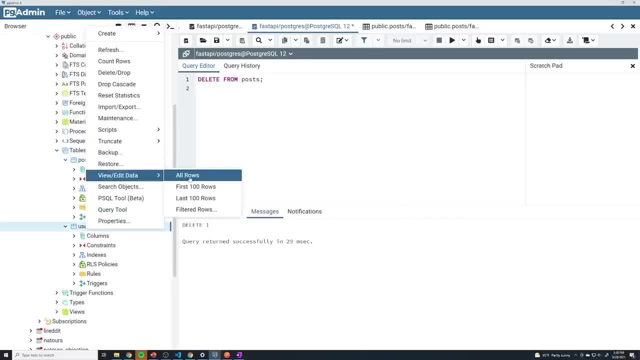 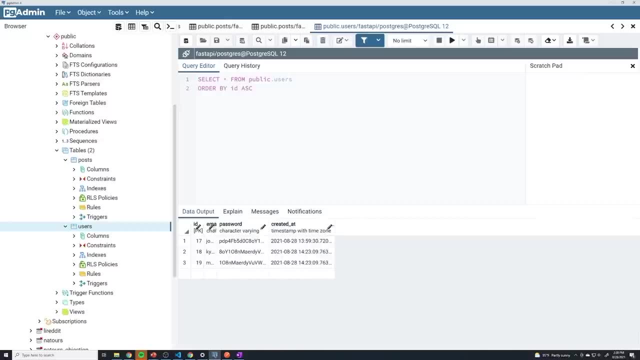 that we're going to go under users. we're going to view all rows And let me clear out some of these. there's too many windows open right, and these columns got a little squished, But right now I have three users. 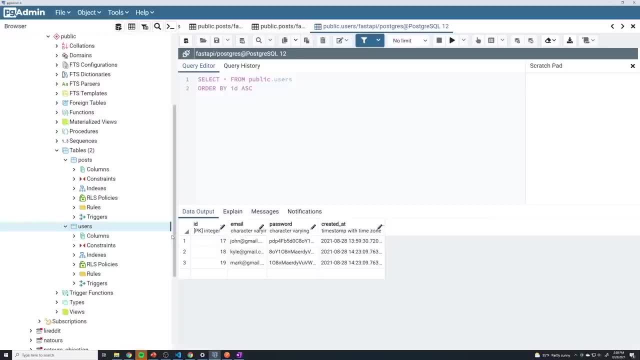 It's got an ID of 17- 1819.. So go ahead and remember that you. obviously your database is going to be different, So just remember the IDs of a couple users And what we're going to do is we're going to go under our posts And we're going to view, edit, And so right now I have no posts because I. 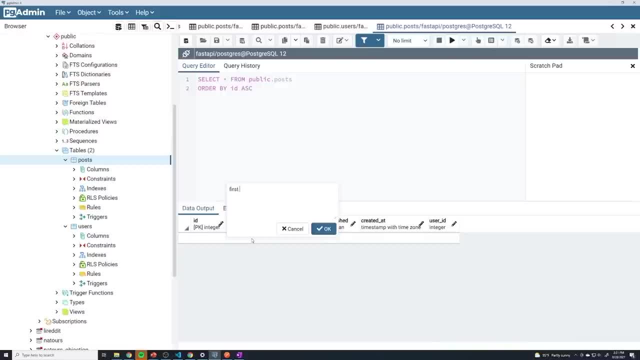 deleted everything, So I'm going to create a brand new post And I'll just call this. that is my first post And the content is just gonna be some random content. I'll leave published blank because we've got a default value. 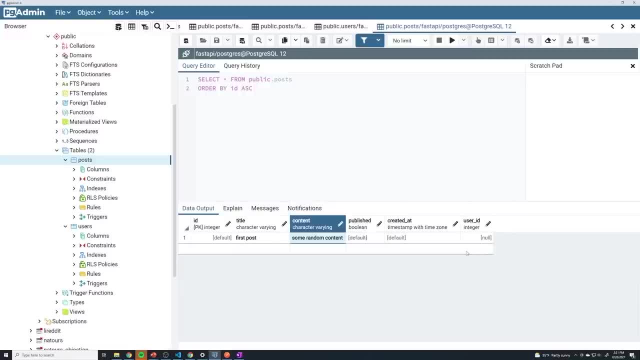 And then right now, if you take a look, we've got this new user ID column. So if I try to save a post right now, take a look at what happens. It gives me an error. It says no value in column. user ID vol violates. 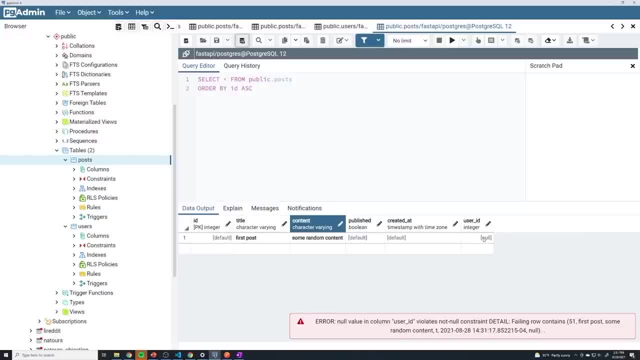 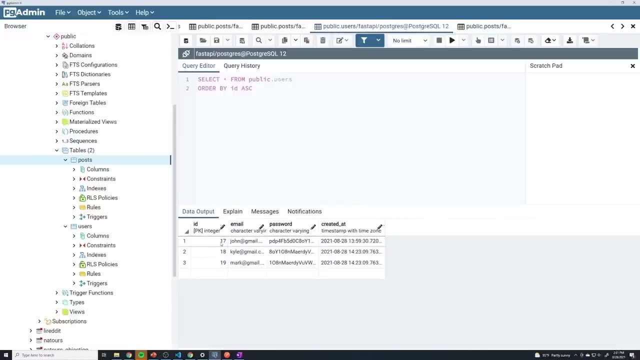 not null constraint. So because we said that user ID cannot be null, we have to provide a user ID. So let's give it an ID And if we go back to users, I can see that there's going to be. I can use 1718 or. 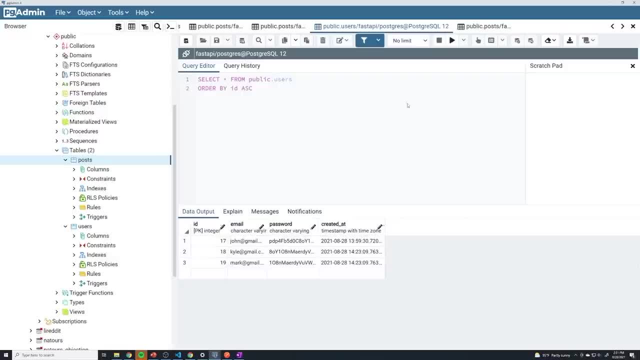 19.. So whatever user created this- I'll just say John created this- we'll grab an ID of 17. And I'll say that this is going to be an ID of 17.. And then, if we save this, look at that we now have a relationship between the users table. 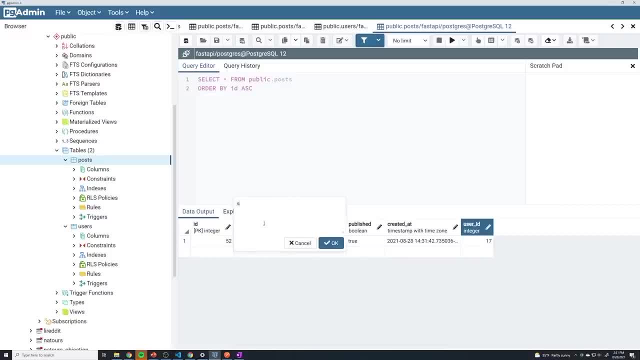 and the post table. Let's create another entry. I'll call this second post, And it's going to have some random content And I'll say that this was created by the user with an ID of 18. And that should work just fine. Now, what I'm going to do now is what happens if I create a post and 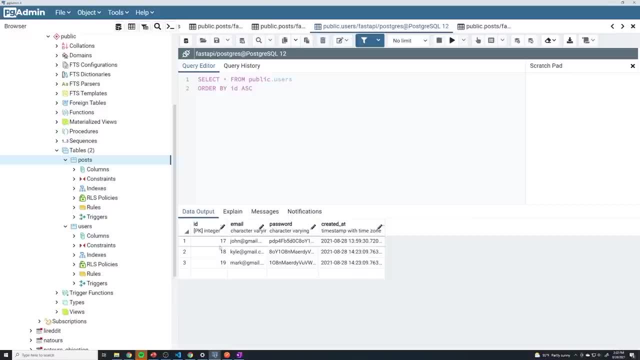 I give it an ID of a user that doesn't exist. So I have IDs of 17,, 18,, 19.. What happens if I set the user ID column to be a value of 20?? Well, let's, let's try that out, So I'll just. 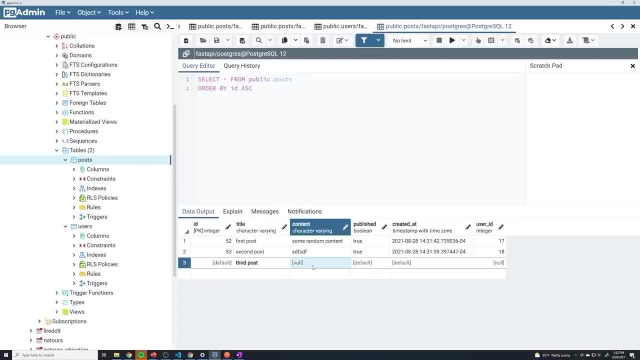 call this third post And we'll set the content to be something random. And if I set this to 20, let's see what happens. I hit save. Look at this. insert or update on table post violates foreign key constraint. there's no user with an ID of 20.. Right, So that doesn't. 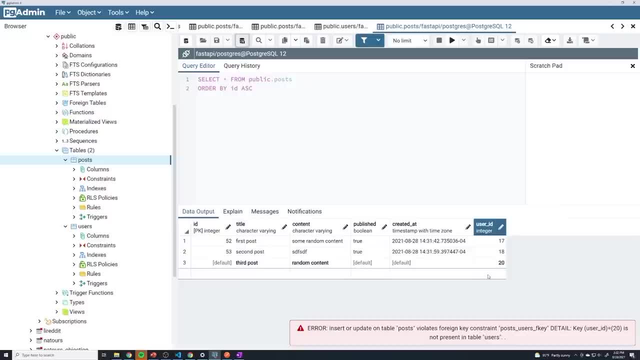 exist in that table, So it's going to throw an error. So that's the magic behind foreign keys that it's going to check to make sure that that user actually exists, And so this isn't going to work. So we'll just set this to 17 as well. 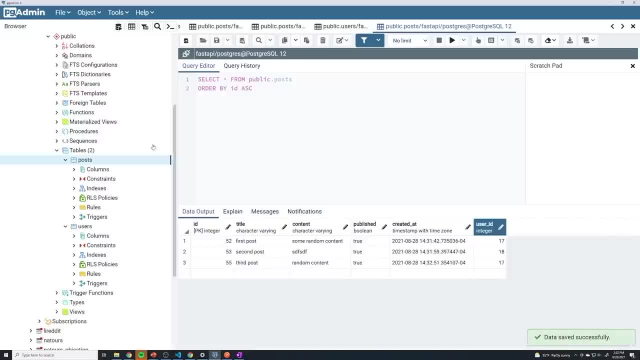 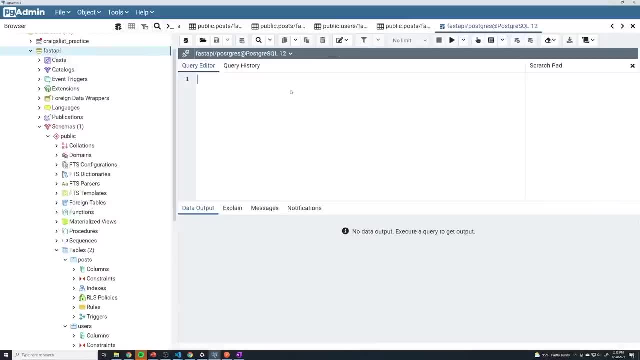 Now save that, Right, And that's it, guys. And when it comes to you know kind of querying these users, right, let's go back to our database And let's just set up a query. Now, let's say I want to get all of the posts created by user 17.. Well, we can do. select. 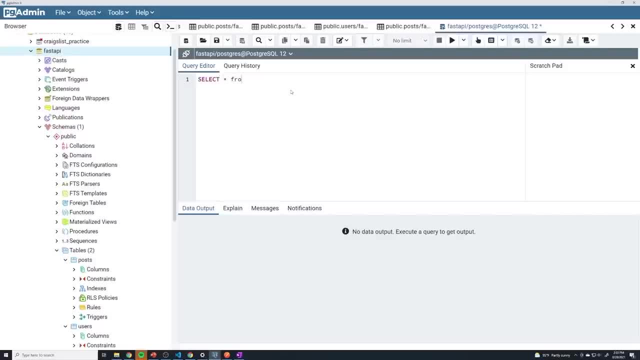 star from posts where and now, instead of you know, searching for based off ID, we grab the user ID column And we set that equal to 17.. So this is going to get me all of the posts that were created by user 17.. I run that you can see that this got the two posts from user 17.. And then, if I change, 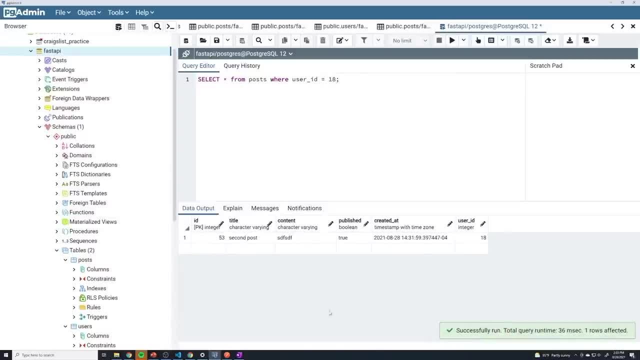 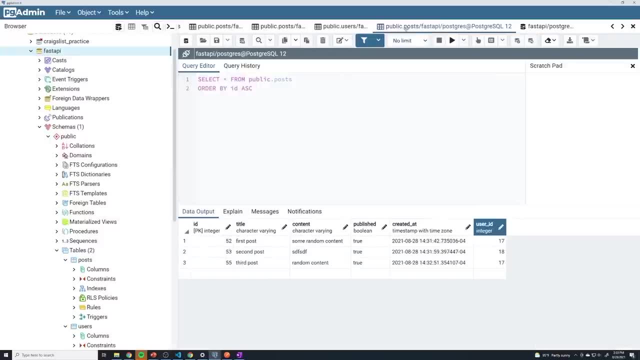 this to 18,. we're going to get the one post created by user 18.. So, from a SQL perspective, right, nothing's really changed. you just specify what column you want to match on and then provide a condition. Now, what I'm going to do now is I'm actually going to set up a query for this, So I'm 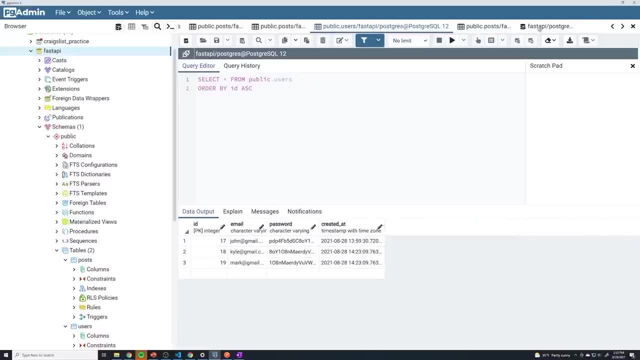 actually going to delete this user. So I'm going to go and just say delete from users where ID equals 70. So we're going to delete john at Gmail And we're going to actually do that here. So I'll say, first of all, select star from posts, All right. so we've got all three posts And I'm 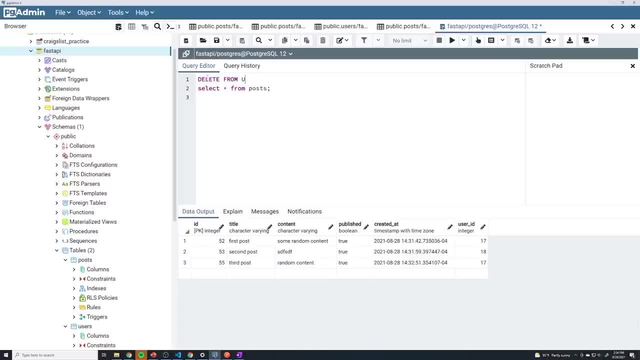 going to run another query, except I'm going to say delete from users where ID equals 17.. So what is going to happen when we delete those users because we have posts that have relationships to them? Well, since we set the on delete to cascade, it should delete. 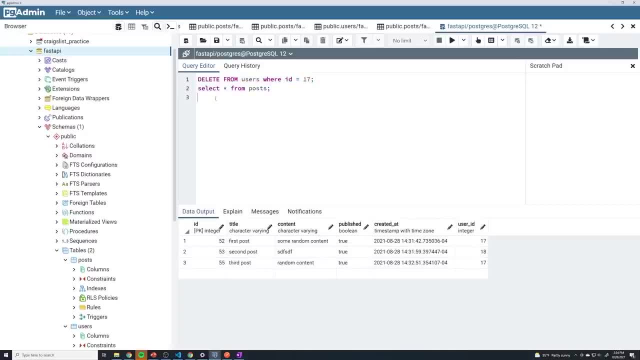 these posts automatically for us. So I'm going to leave this down here. So it's going to run another query So we can see exactly what our table looks like after we delete this user. And so if I run this, you can see that when I run a select star from posts, there's only one entry. 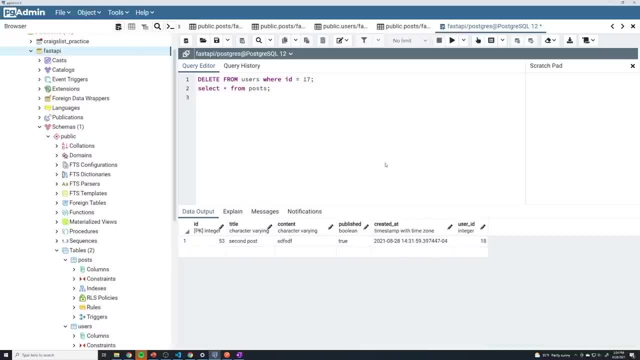 left, And that's the one with the user ID of 18,, because it automatically deleted all of the posts created with an ID of 17.. All right, and so, from a database perspective, I think this is all we really need to cover for now. Eventually, we'll start taking a look at joins, which is how to run. 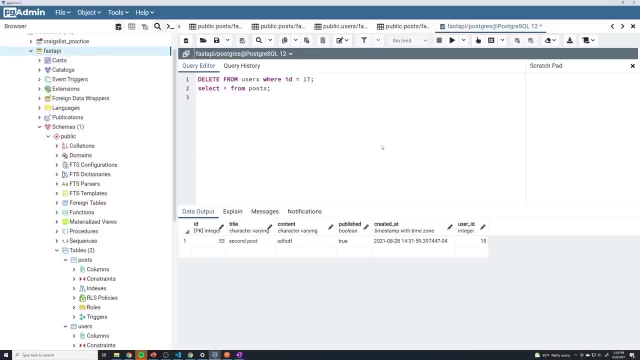 these complex SQL commands that allow you to jam the columns of multiple tables into one result to make it a little bit easier to retrieve information. Because right now, if I, if I try to get all of the posts, you know, like every single post in my database, right, it's just going to give me the user ID. But if I need 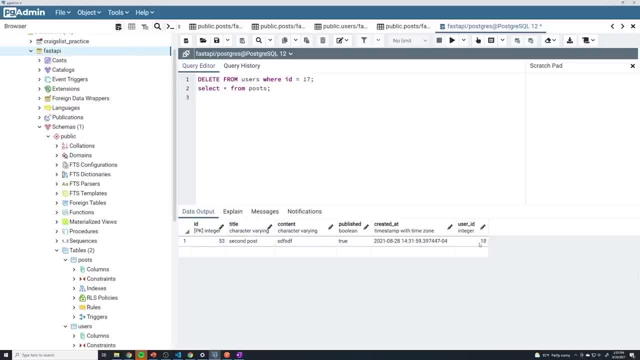 the information about the user, like what's the name of the user, what's the username or the email, then I would have to individually query the the IDs of these users. So I'd have to go, then I'd have to do, you know, a select. oops, make sure I don't delete anything. I'd have to. 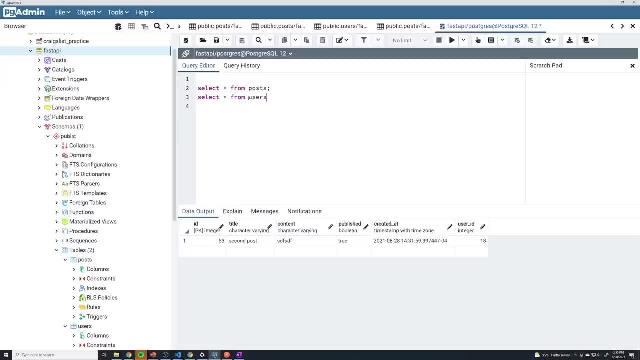 do a select star from users where ID equals 18.. And I have to do this one by one for every single user So that I can get this specific user. And so that's when we start to make use of things like joins. But that's a little ahead of us at the moment And that takes a little while to explain. 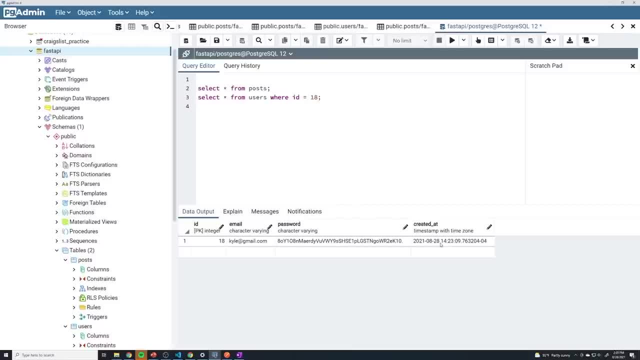 So we're going to come back to that. But before we actually kind of move on from this database side of things, because we pretty much covered everything, we're going to delete that column for now because we're going to make sure that SQL alchemy actually sets up all of these constraints for us. 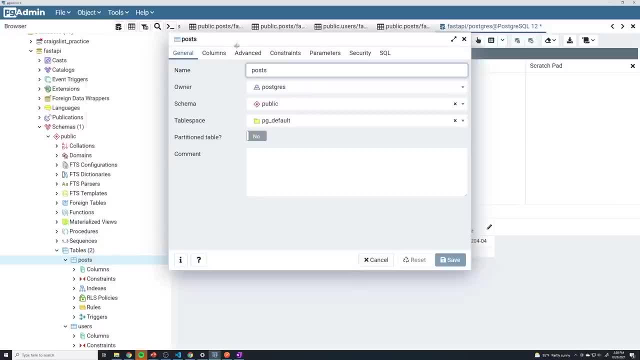 automatically, so that we don't manually have to do it. So let's go to our properties, go to columns. we can just delete this column And then I think this should automatically delete the foreign key. it does not delete the foreign key. 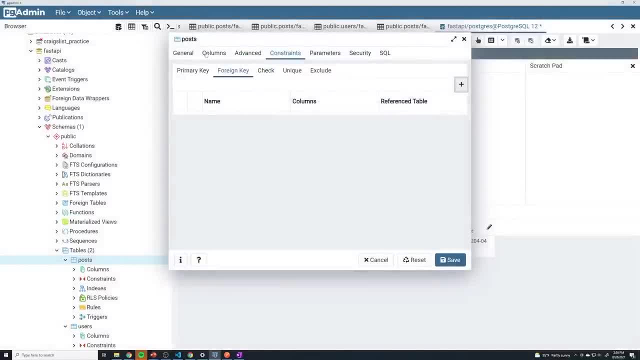 So make sure you delete that as well, And then we can save that And it looks like there's throw in an error. So let me cancel out of that And I think we're gonna have to do this in a two step process. 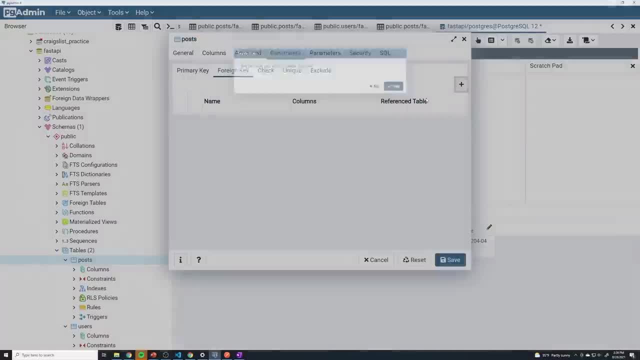 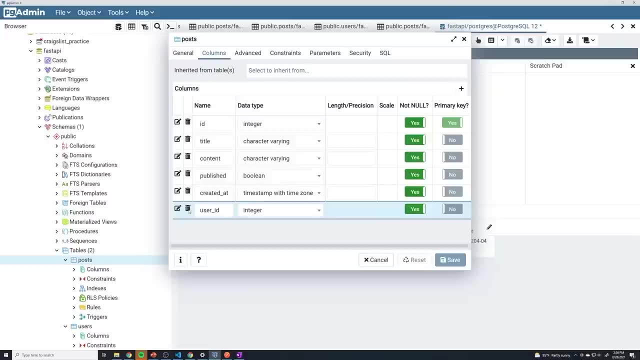 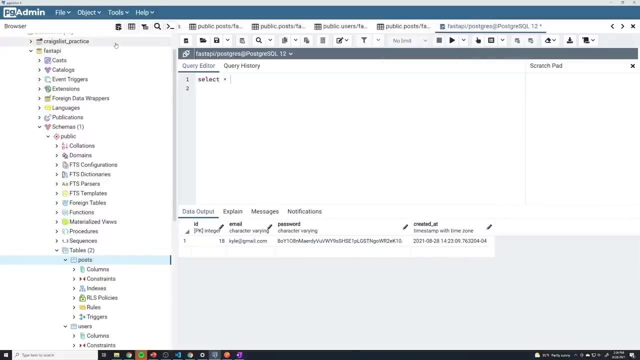 So we'll say constraints, we'll delete the key first We'll save that and then properties will delete the user ID. There we go. And so now, if I do a select star from posts: right, there should no longer be a user ID column. 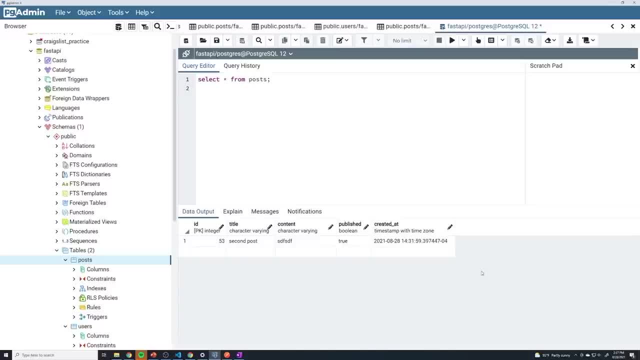 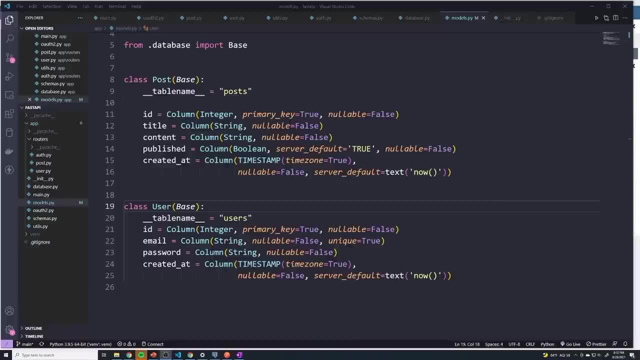 So this put our database back into the state it was in before we started playing around with it. So now that we know how to create and set up a foreign key within Postgres and PG admin, we're going to see how we can do this through code, using SQL alchemy, Because 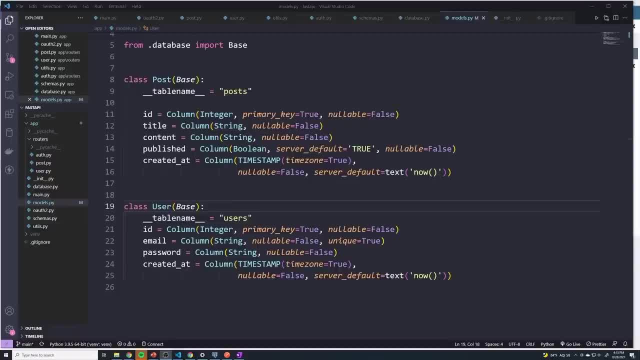 ideally, since we're already using SQL alchemy to generate all the tables, generate all the columns for each table and all the different properties, we should also set it up to generate the foreign key for us as well. So we're going to go to the models that py file. this is: 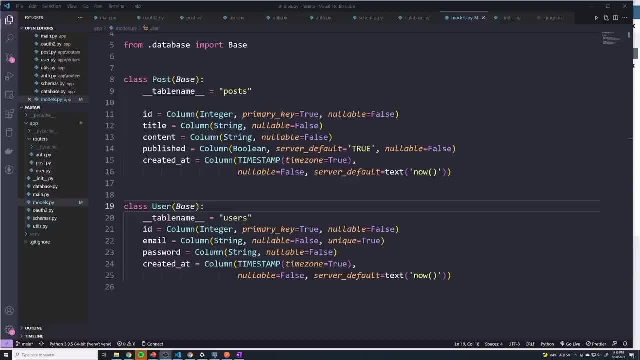 where we define what the tables are going to look like with the different classes, And we're going to add a new user ID or owner ID column to the post class And that's going to create a specific column within the post table And so we can just go here and you know, call it owner ID, user. 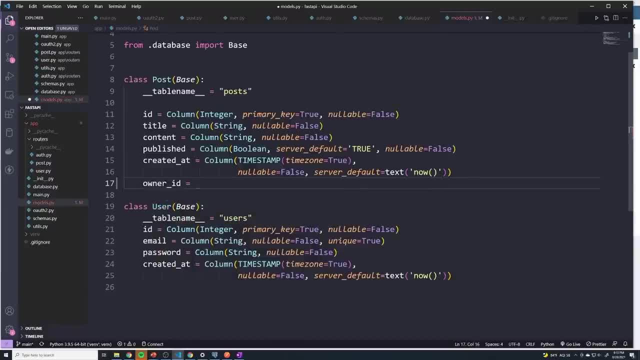 ID, whatever you want. I'm just gonna call this owner ID And this is going to be column. And then here we have to specify the data type of a column And, as I mentioned, the data type should match up with whatever the data type of the foreign key is. So, since 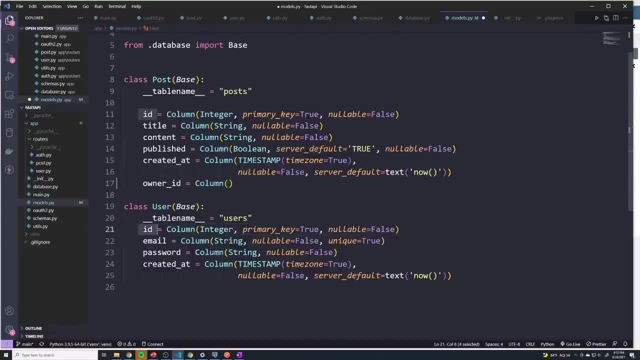 this column is going to point to the ID column of the user table. it should match up with whatever is here. So since this is integer, this has to be integer as well. Then, to set up a foreign key constraint, you just type: 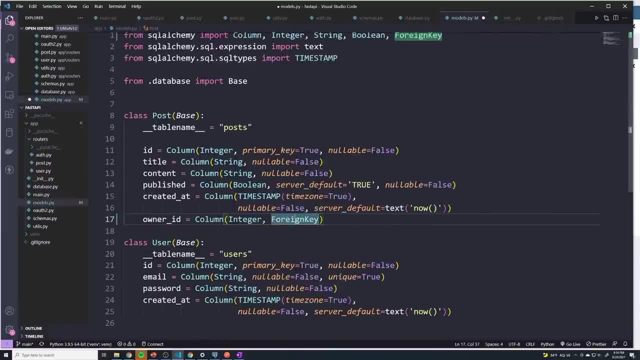 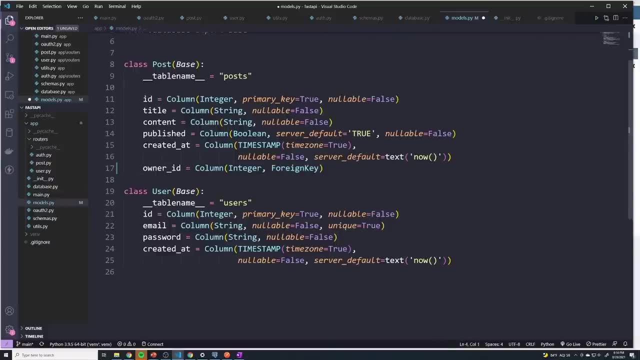 in foreign key And then go ahead and auto import that. if you don't know where it's getting imported from, it's going to get imported from SQL alchemy. So if you didn't automatically do it, you can go ahead and just manually type that out And then there's going to be. 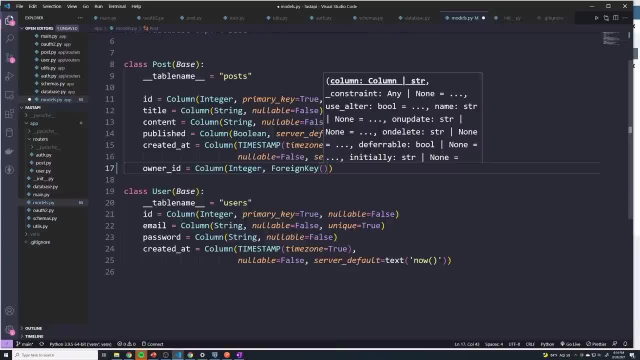 two fields that we're going to pass in. So the first of all, we have to pass in the exact column and table table and column that we want to reference. And since we don't have that, we want the users table and then grabbing the ID column. And so your instinct would: 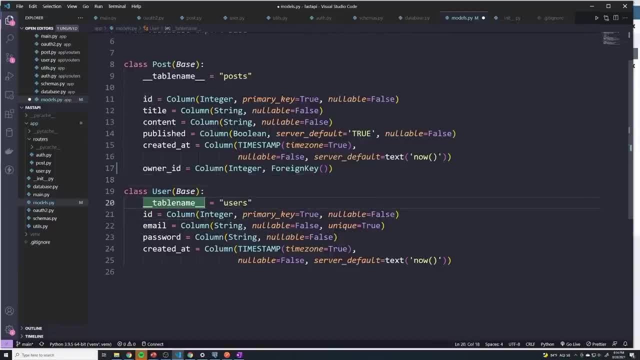 be to use the class name, but we don't actually reference the class name. Instead, we want to reference the table name, So it's going to be lowercase in this case. so you say users dot. and then what's the column name? it's called ID, So we say dot, ID. 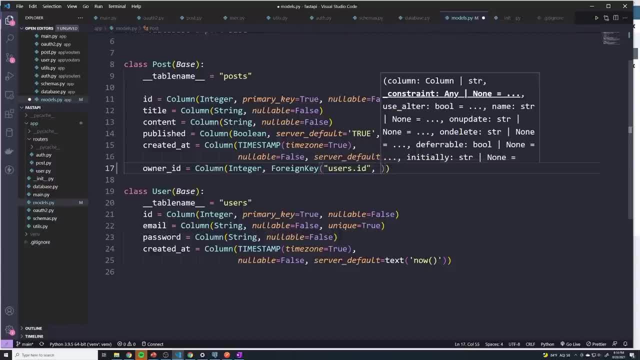 And then the second thing we need to do is, if you recall, we have to set up what the policy is for when we delete the foreign key or the parent table, And so we always used a cascade That if the parent object gets deleted, all of the child object objects get deleted, as. 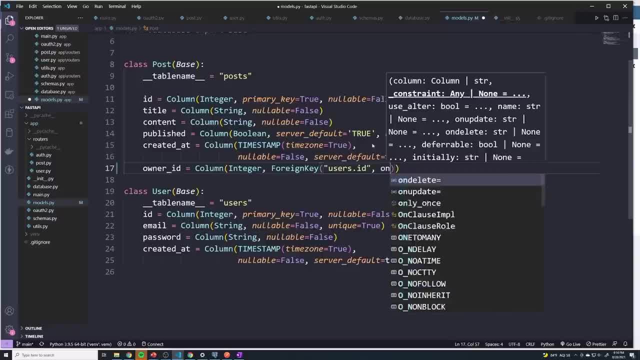 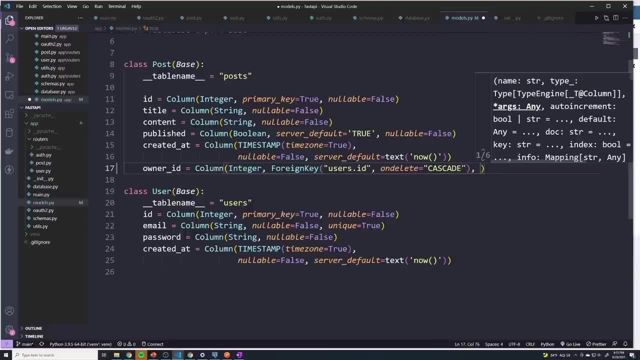 well, So we can do that through SQL alchemy as well, And we'll say: on delete equals, And then we just say cascade, And then, finally, we want this field to be nullable, equals false, So it has to be filled in. All right, And now, if we save this, restart our application. 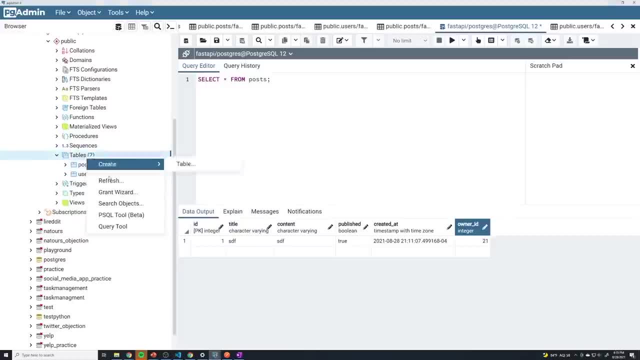 we'll take a look at Postgres And if I actually refresh this field, we'll click on it And this is actually an old, an old panel. So I'm going to remove that And then, if I just do, we'll go to our post table, go to query tool. I'll say select. 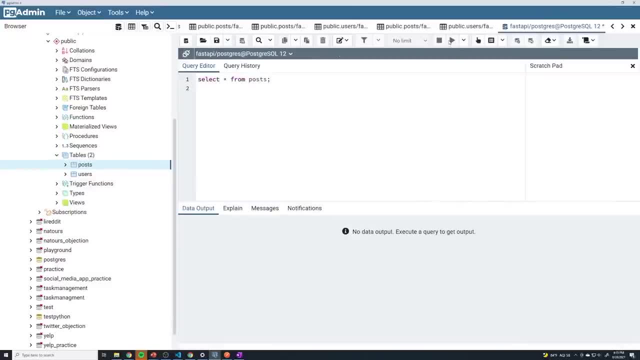 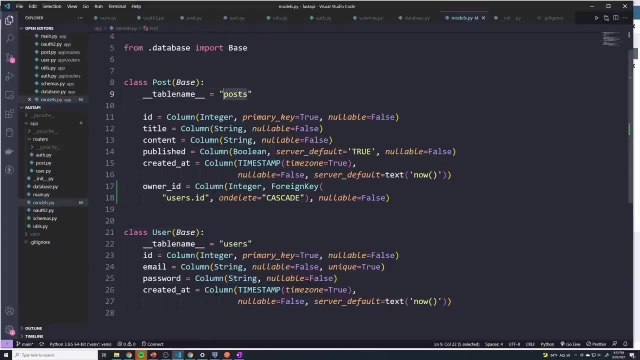 star from posts Run that you can see that there is no actual owner ID column, And so the reason for this is that SQL alchemy, when it, when we start our application, SQL alchemy will check to see if there's a table called posts, And if there is, I'm sorry if there's. 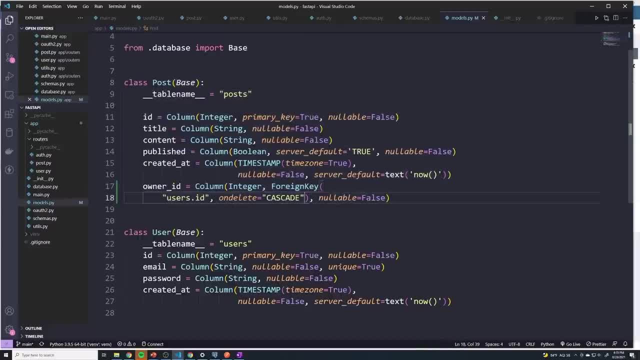 isn't? it's going to then create a table based off of these rules. However, if there's already a table named posts, it's not going to do anything. So if we update any properties for a pre existing table, it's not going to change that. That's not exactly what SQL alchemy is meant for. Instead, 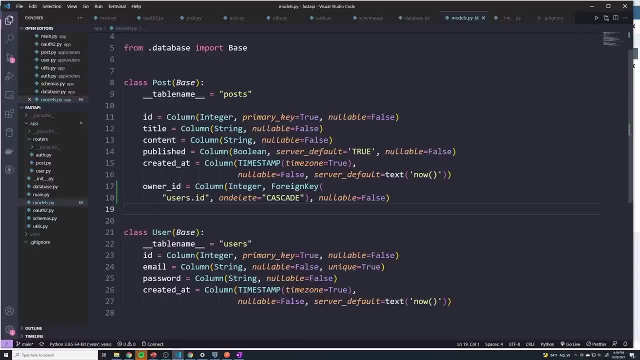 we would have to use a database migration tool, kind of like Alembic, which we haven't covered yet. So instead, for now, what we're going to do is we have a couple of different options. we can manually just do it, go into pgadmin, add the things yourselves, Or we can just take the 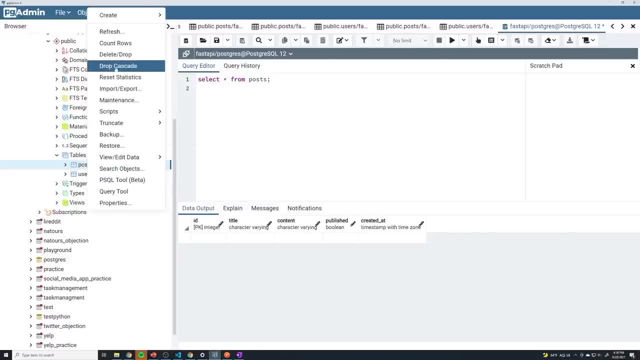 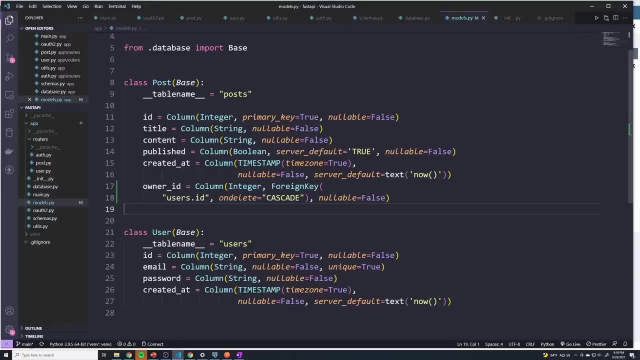 easy way out, Since this is a development environment, we can just drop our post table- And that's one of the luxuries of working in development- So you can then hit save again, and that's going to cause it to restart the applicant, the application, And then, if we go, 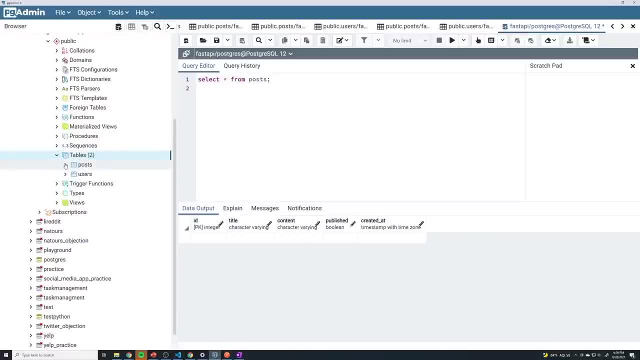 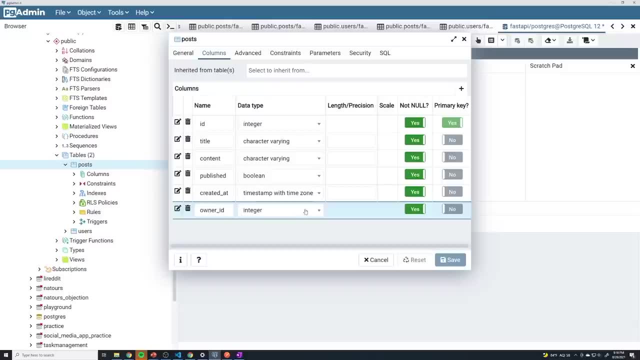 to Postgres and we just hit refresh. it's going to create a new post table And then we can go into properties And we'll go into columns. And we now see that we have an owner ID column which is going to create a new post table And then we can go into properties. And we now see 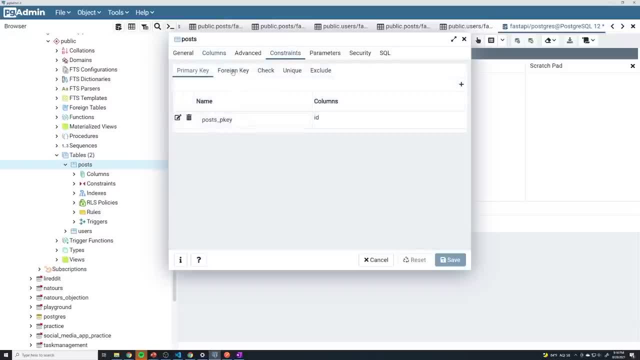 that we have an owner ID column which is set to not null. that's good. And then if we go to constraints- foreign key- you'll see that we've got our foreign key And you can take a look at the details down here. And the main thing I want to check is for actions we do have on delete. 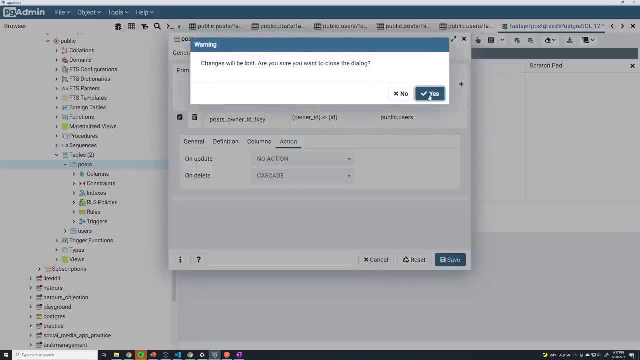 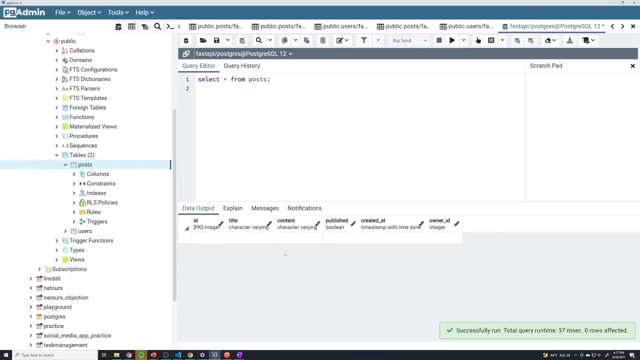 cascade, Alright, and so now that we have everything set up, if I just run this query again, we should see the owner ID show up. So let's create a few entries, And before I do that, I need to make sure that I actually have some users, because I kind of went in and deleted a few. 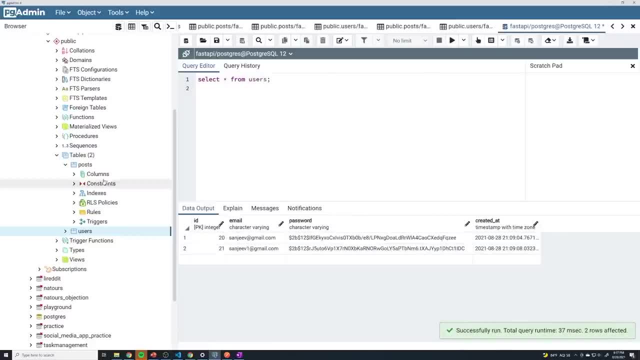 users. So I've got two users with an ID of 20 and 21.. And so what we're going to do is we're going to make sure that the foreign key points to one of those IDs. So we'll grab a post. I'm going to just 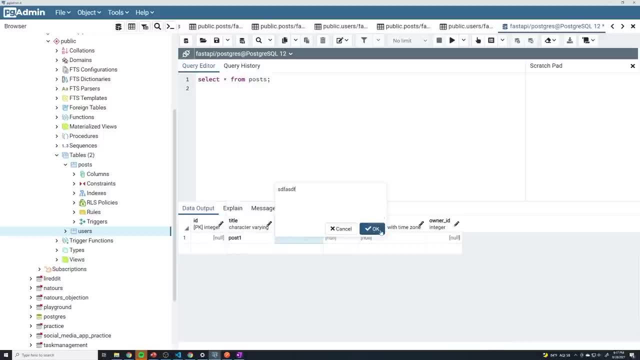 set this to be post one as the title- And it's going to be some gibberish- And then we can set the post the owner ID to be the ID of a user that we already have in our database. We'll save this. 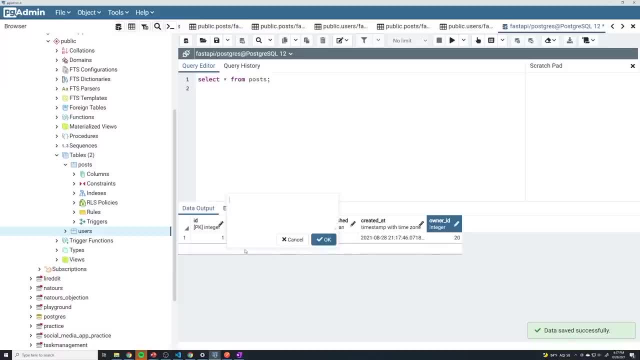 and we can see that it's successfully created. Now, if I create a new post, and this time leaving the owner ID blank, if I hit save, you can see that it throws an error because this can't be set to null. And if I try a ID of a user that doesn't exist, like 57,, 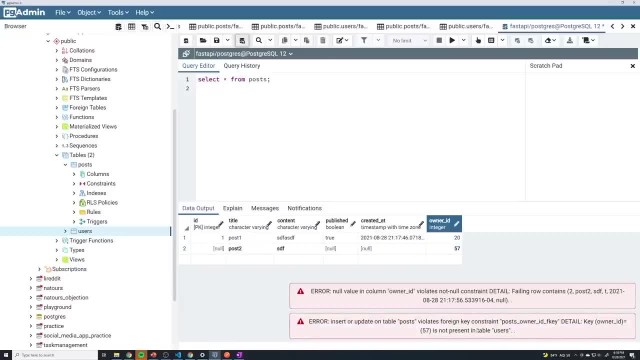 it should also throw an error. And so it's saying that, hey, the owner ID of 57 does not exist in the users table, And I'll just change this to 21.. And then it should work. Great, Now let's quickly. 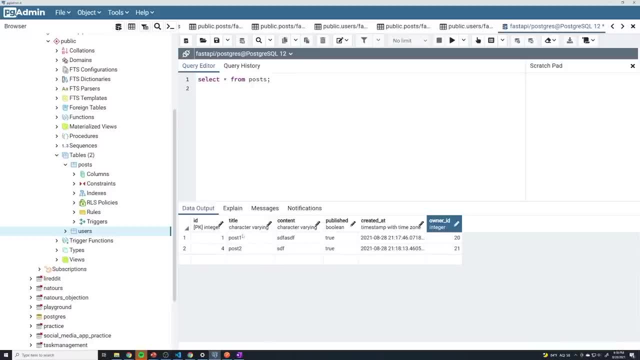 check out the on delete functionality just to make sure that it works, And what we're going to do is: let's go to. well, I'll just run the query right here, We'll do delete from and we'll say users where ID equals and we're going to delete the user with an id of 20.. So, if everything works, 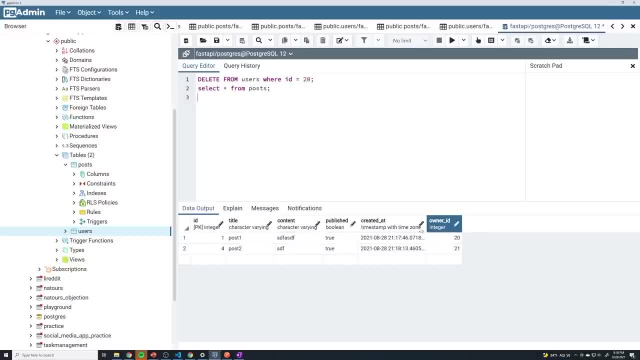 we should see just this entry also get deleted in the post table because the owner is as an ID of 20.. And since that owner is going to be deleted, then we should only have this one left. So if I run this, it, we can see that the one with the owner ID of 20 is now deleted. All right, and so that kind of handles the. you can see what happens if you fix the link and then I'll just take that and I'll just get an ID of 20 to the post table. Also, we should have a. You can see where the owner ID went. So that's. 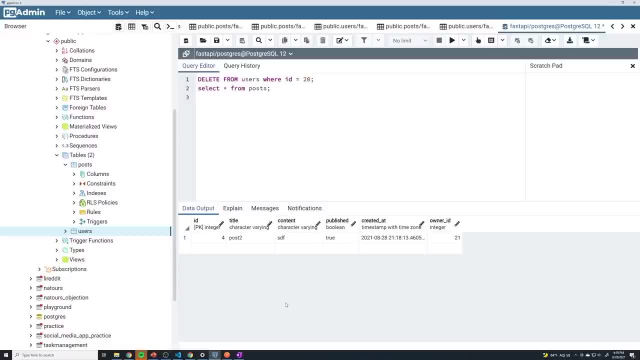 of the database side of things At this point. if you try to test the rest of your application, you're going to probably run into a couple of issues. But that's just because you know we've hard coded our schema to match a certain you know number of properties. And so, since 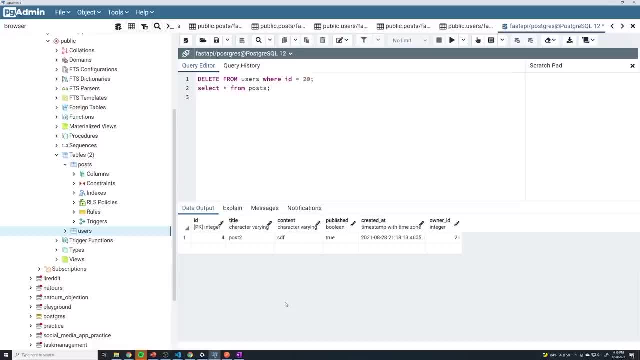 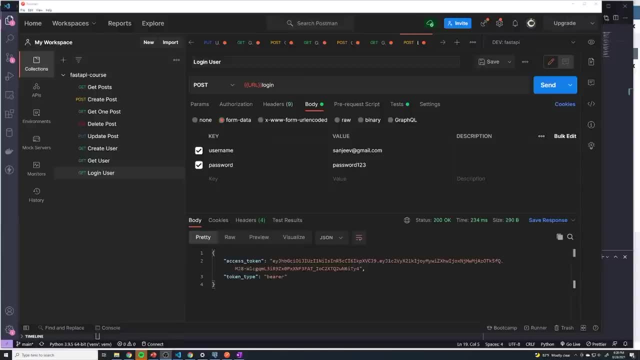 we've added this new property to our posts. it's going to throw a few errors, So we're going to have to update a few things in the next video, But you'll see that updating your schema is very simple. With the changes we made in the last lecture, it's inevitably 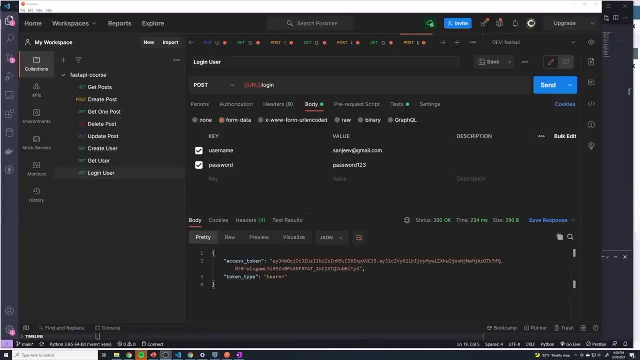 going to cause some issues with our application. So there's gonna be a few things that we have to update within our app, And so let's just quickly run through a couple of our requests just to see what they look like, see what changes we need to make, And so, if you haven't, 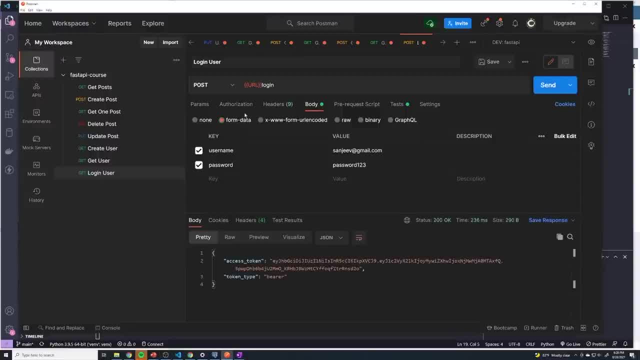 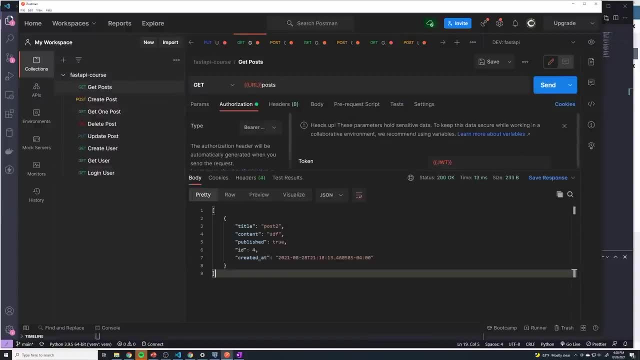 already done so log in a user, And so once we're logged in we should update the variable And now we can retrieve our posts. So if I hit send here, you could see that we retrieve all of the posts in our application. I just have one in this case. But the first issue. 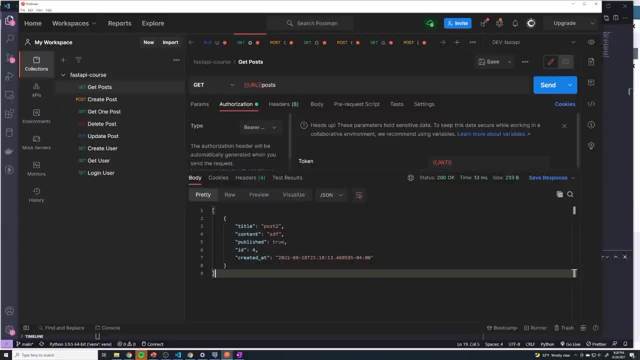 that I see is that we're not returning the owner ID Right? This is a brand new column And I would expect this information to get sent out to the user. And the reason that I would expect this information to get sent out to the user. and the reason 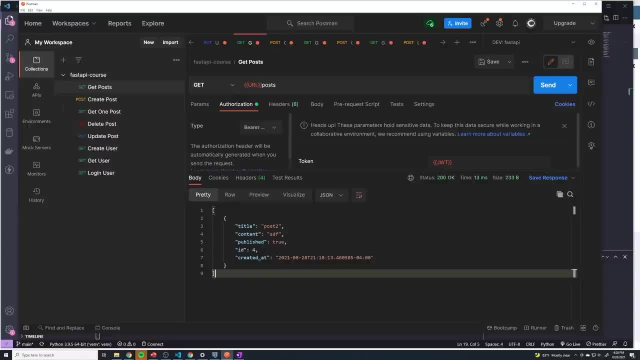 why it's not included in here is that we have to actually update our schema, because our schema probably doesn't have that owner ID, because we never added that in And you might be thinking, well, do we actually need to send it? Yeah, I think it makes sense for. 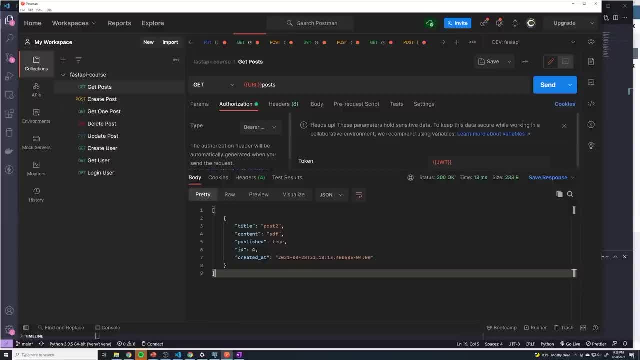 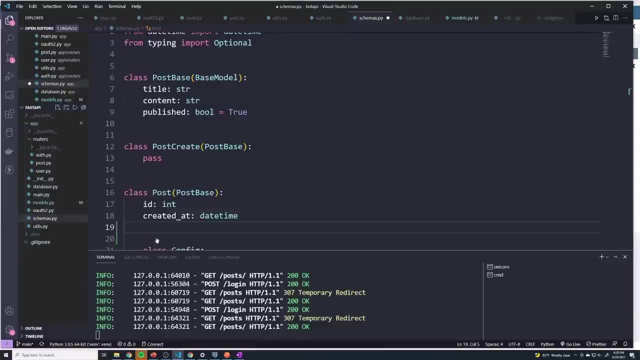 us to send it, because any, any application, the user should know who creates a post. So ultimately they're going to have to get that information, And so we should provide the owner ID. So let's go to our code And if you actually go to the posts, router and 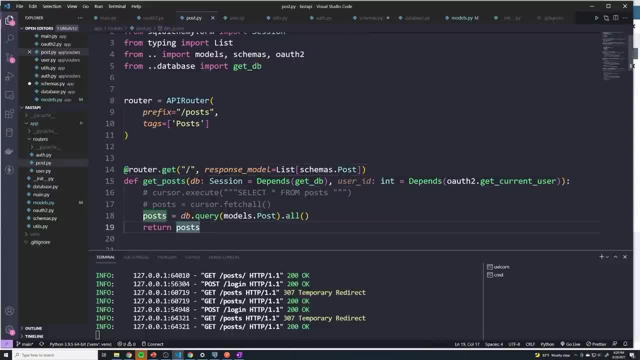 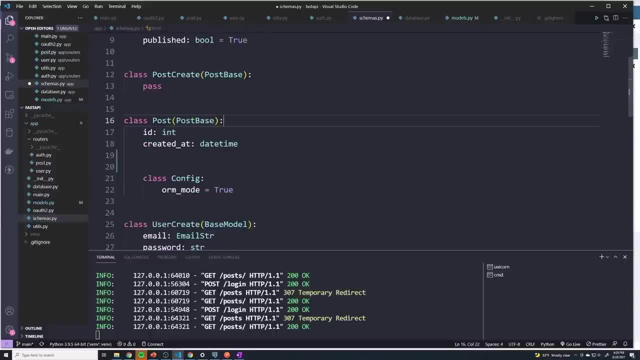 take a look at the get all posts, you'll see that the response will be the same as the response model is going to reference schemas dot post. So let's go to schemas dot post And you can see that this is what we're using to return. This is the schema that we're. 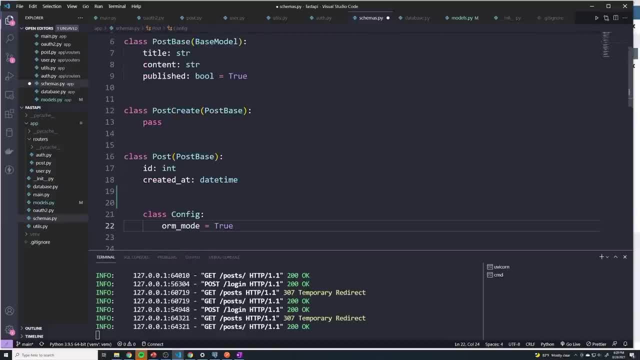 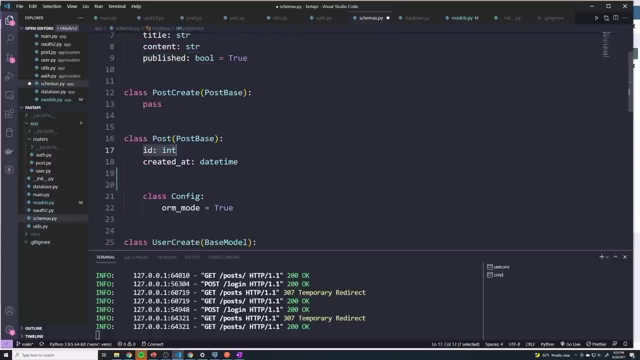 going to use for returning posts to a user, And so this actually inherits from post base. So post base has title content published, And then we extend that and we're going to add the ID which gets created at the database level, as well as the date and time or the. 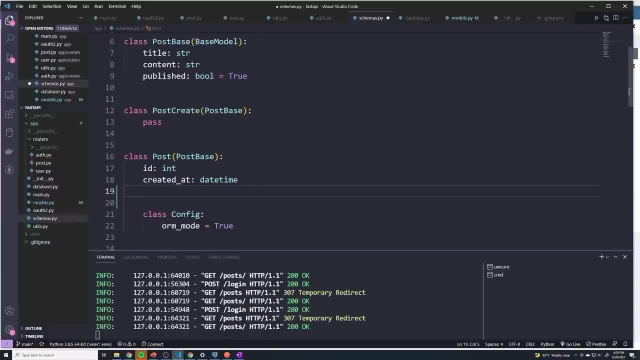 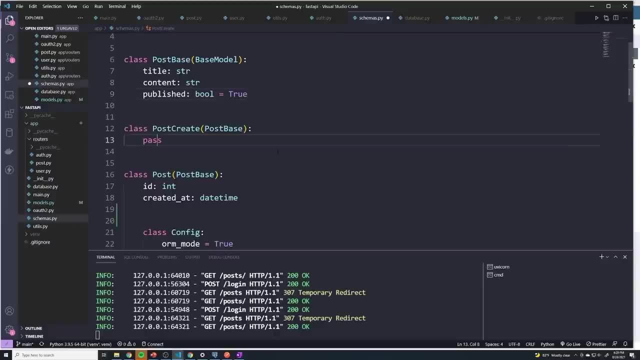 created that field which gets added by the database, So we can add it here. However, I'm sure you're thinking: well, could we add it at post base? Should we add it, post create? Well, let's think about this, The first thing that we have to think about. 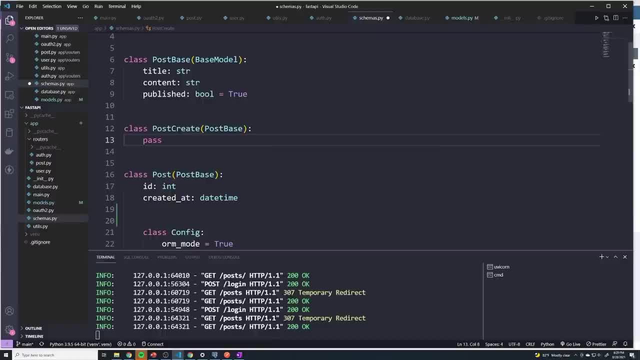 is, when we create a post, should we be passing in a owner ID? Well that, we 100% absolutely could do that, And that actually does kind of make sense. So in that case, if we did want it to be available or require it for creating a post, then we would add it under. 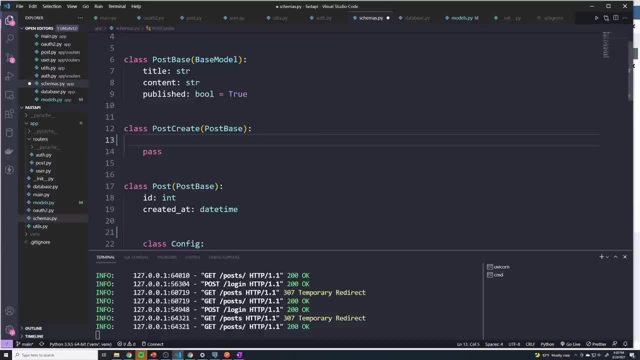 post create here as well, Or we could just add it under post base so that both of them inherited. However, what we're going to do is we're actually not going to require the user to provide the owner ID. Instead, what we're actually going to do is we're going to let the the logic of our route. 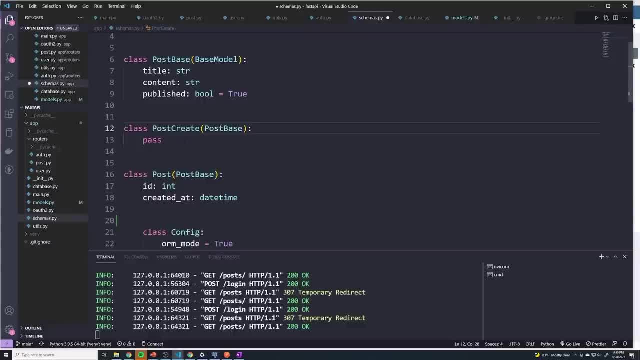 to actually just grab the ID from the token and then use that as the field. So we don't actually need the user to pass that into the body. So we're not going to. we're not going to use that field or apply that field to either one of these classes, we're just going to. 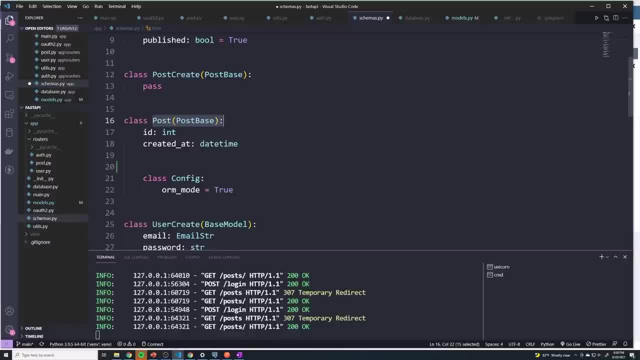 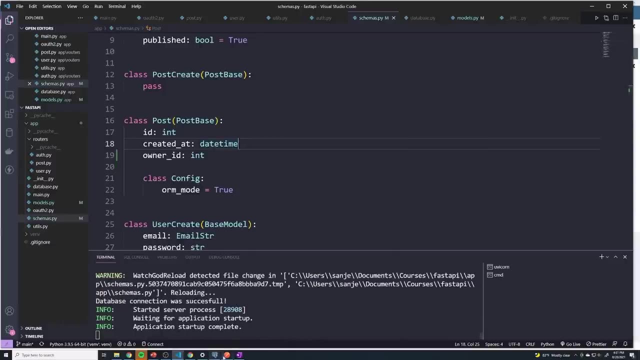 do it for the post class, which is the one that's responsible for sending the post out. So I'll add a column here And we'll call it owner ID And I'm gonna say that this is going to be a type of int. Alright, let's save that And let's see if that makes a difference. 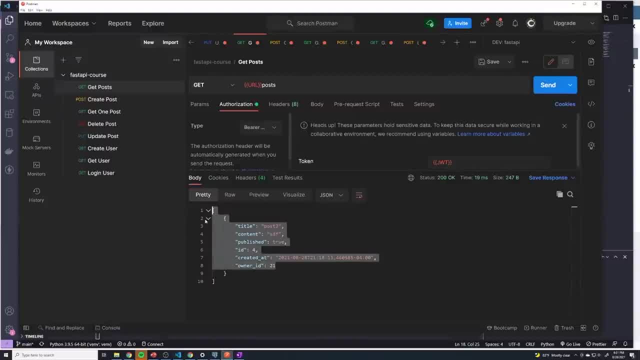 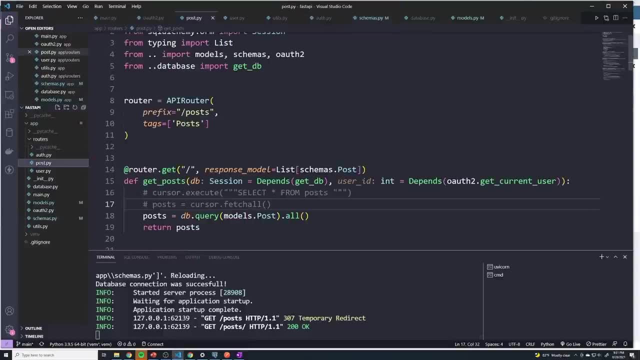 So let's hit send And so now we can see that we get the owner ID And that's really all the changes we have to make. So if we actually go to get one post and we look at our code here, if you look at the postpy for getting an individual post, you can see that we're 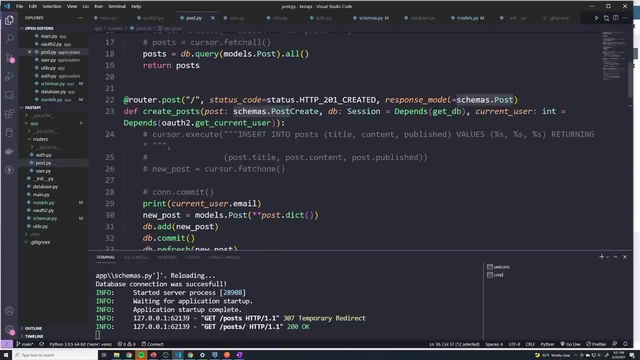 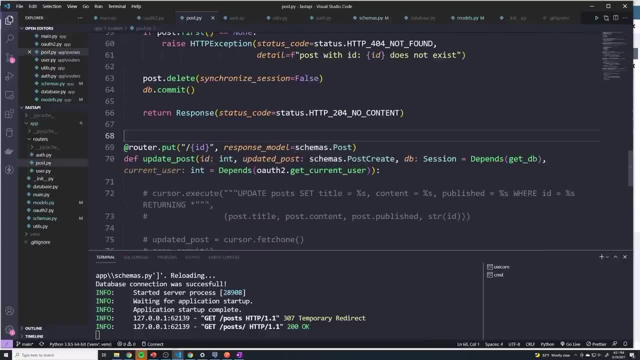 returning the same exact model. And if we take a look at creating a post, we return the same model, So all of those will be updated accordingly. And same thing with the update post. the update post also uses schemas dot post. So since we're using the same schema, 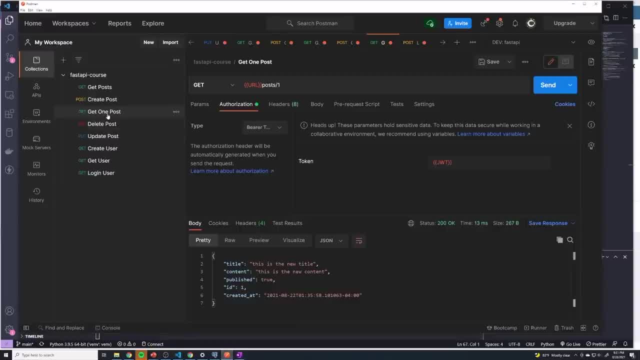 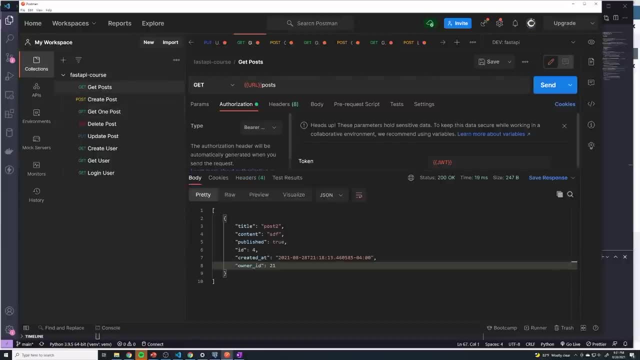 for all of them. we don't have to do anything else And we can just quickly test that out. So I'll do get one post And I realized we have to actually get what was the ID. ID is four. So we're going to update this to be an idea, for you can see that we now have the 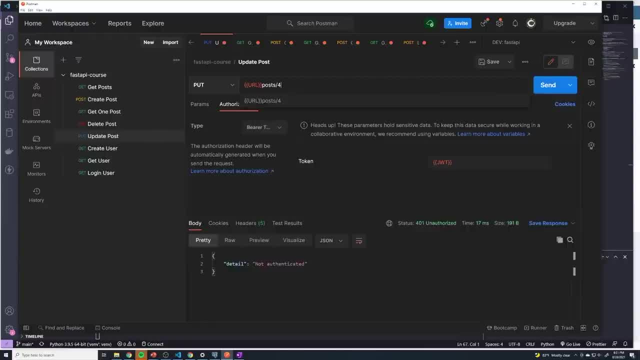 owner ID there. we update it Right, we can once again get the owner ID And at that point it looks like everything else is good. However, if we go to create posts real quick and we create a post right, we get a crash actually. So there is an issue with creating a post. 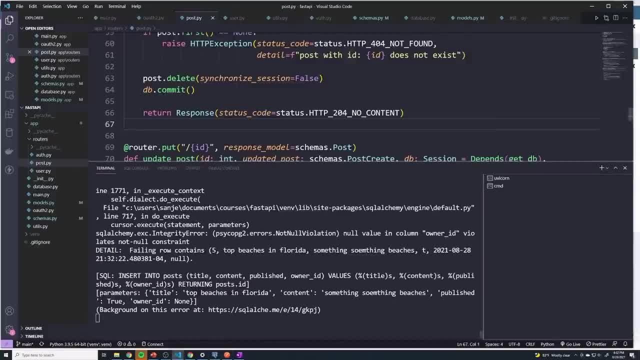 And I'm sure you guys can guess exactly what it is. Take a look at the error When we try to create a post Right, it's saying there's some kind of SQL error And it says there's a null value in column owner ID. And that makes sense. And that makes sense. 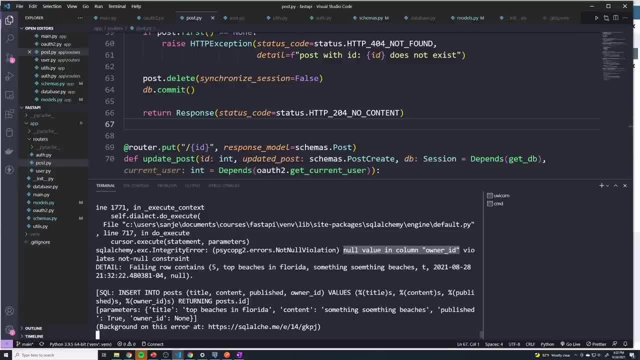 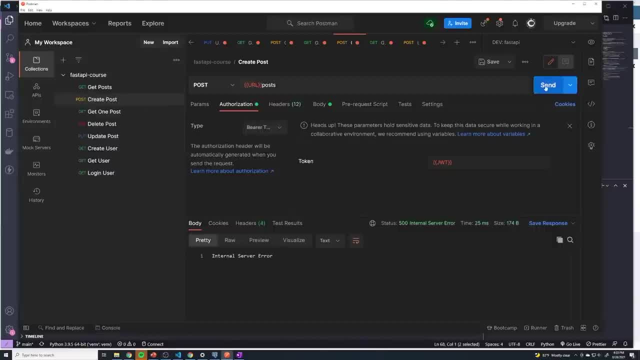 So we'll actually tackle this in the next video And you'll see that it's going to be pretty straightforward to actually get that resolved. So in the last video we learned that the create post functionality is broken now because if I try to create a post, you 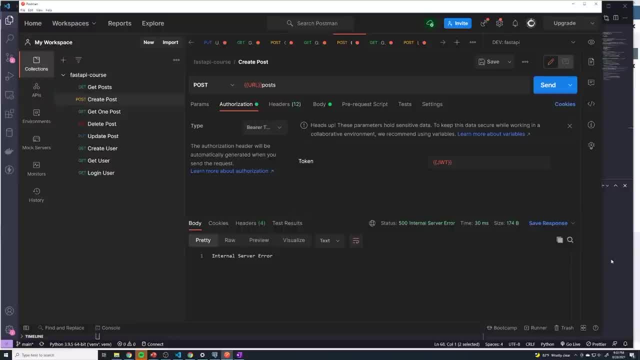 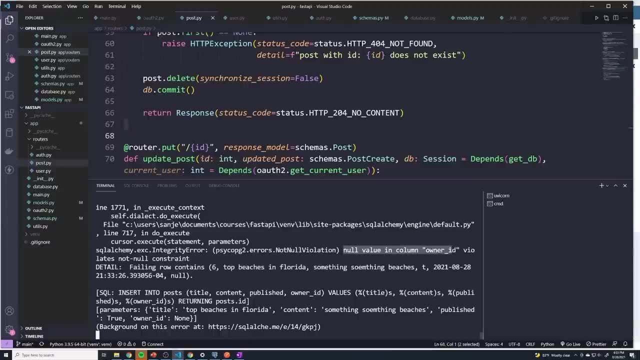 can see that it sends back in a 500 status code, And if we take a look at the logs we can see that it looks like there's some issue with the sequel And it's saying that the null value in column owner ID violates the not null constraint. And so, looking at our model, we obviously 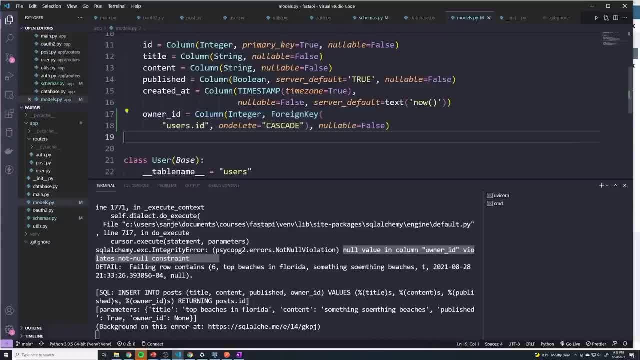 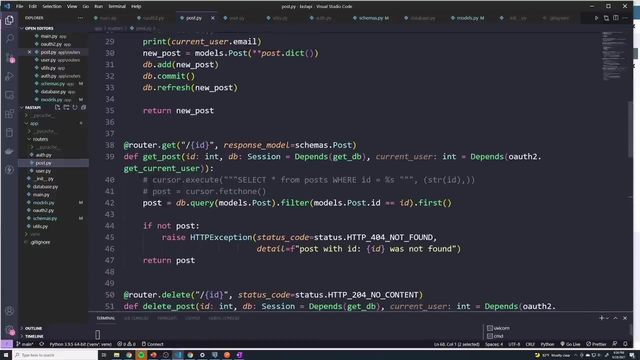 set the owner ID right here, And this is set to be nullable, false. So we actually have to provide who the owner ID is for this new post. So how do we do that? Well, let's go to our post path operation And let's go to the create post path operation, And so it's. 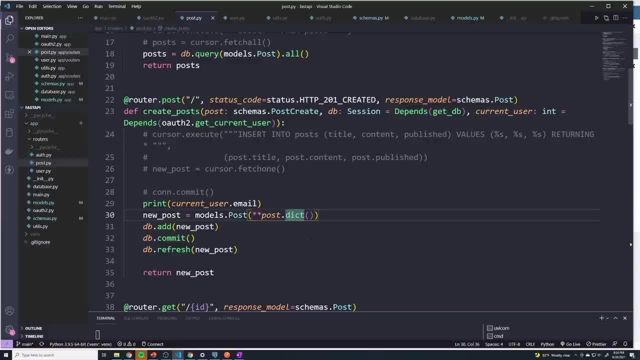 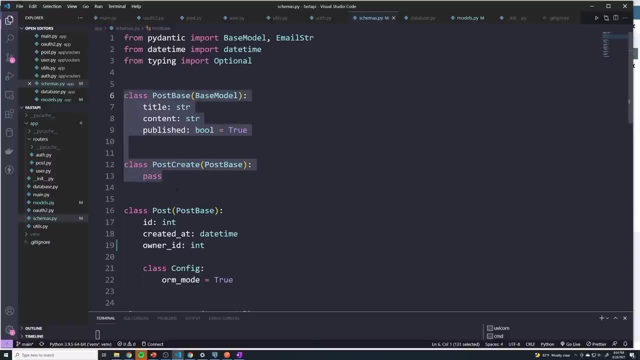 right here, And so nowhere in this code are we actually providing a user ID or owner ID into this new new post that we're creating. we're just grabbing the post which comes from post create the schema And if we look at that schema, you can see that we do not provide a owner. 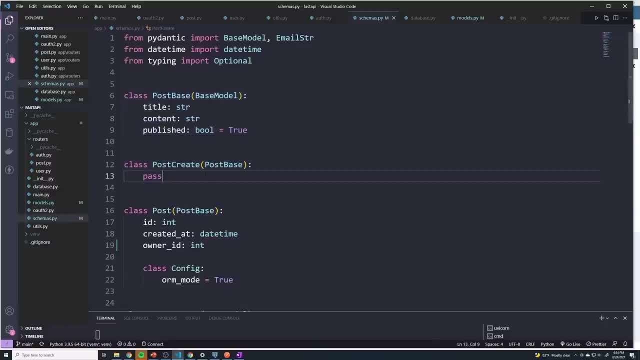 ID And, like I said, we're not going to actually pass the owner ID into the in the body. what we're going to do is whoever is logged in and creating the post should automatically be the owner right. If you're logged into Twitter and you post something, Twitter knows. 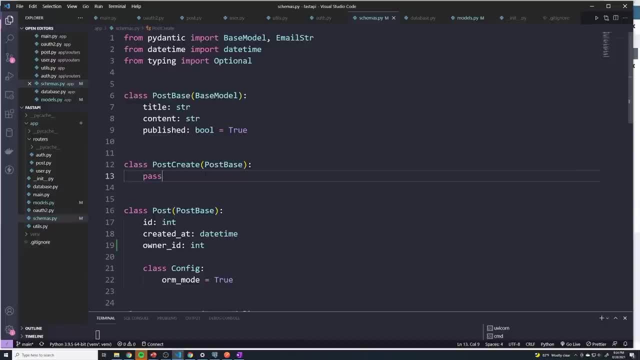 that you're the one creating the post. So whatever ID is associated with your account, it's going to set that automatically, So we shouldn't have to pass that in the body. we should automatically retrieve it from your authentication status. So within post right. 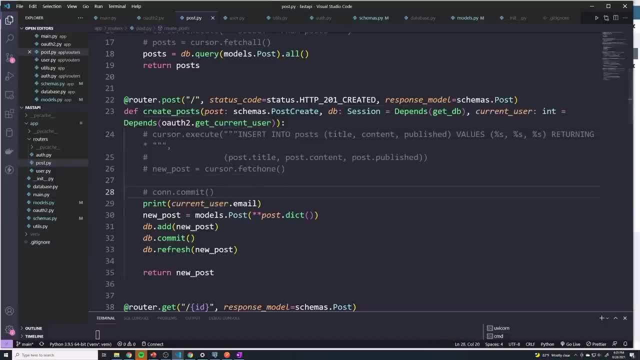 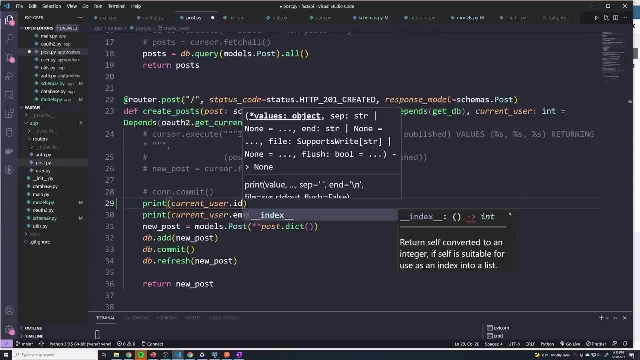 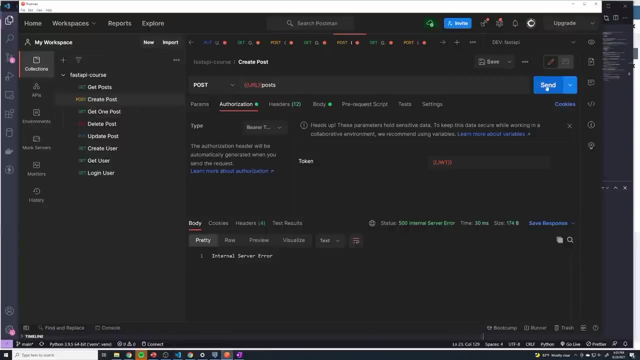 you can see that we have the current user And so we should be able to get the current user or the user's ID. So if I do current underscore user dot ID and we can remove this kind of need the email, And if I tried to create a post, it's still going to error out. that's okay, I just want. 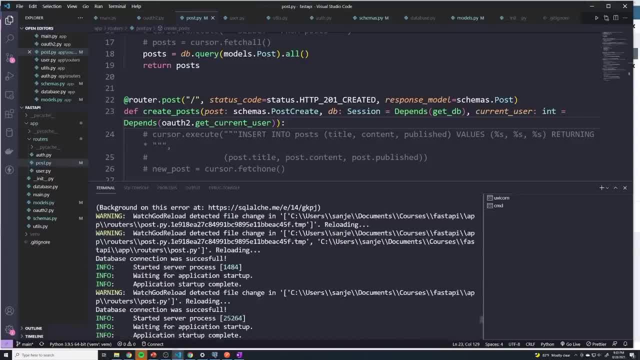 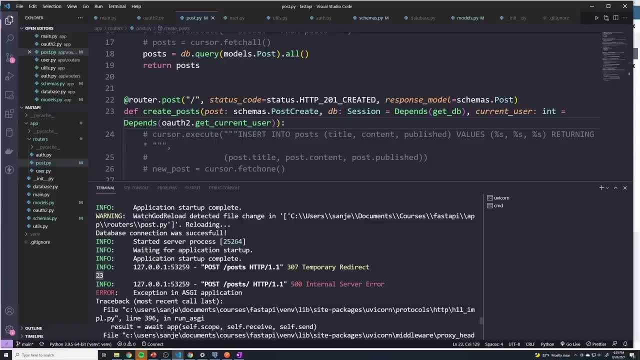 to see what it prints out though before the error, And you can see we got a lot of errors, that's okay. And you can see that it printed out the ID of my user, which is 23.. And just to double check that that's actually my user. I'm going to select star from users. 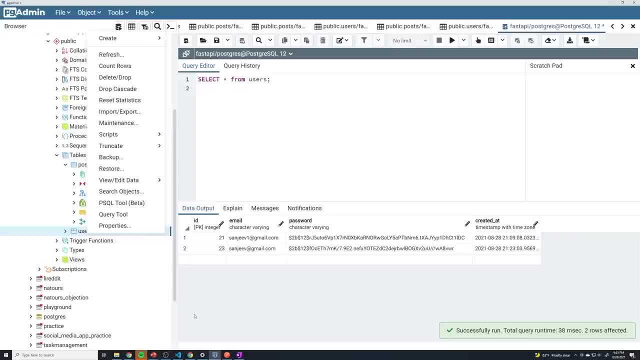 And you can see that 23 is Sanjeev at Gmail. So we could just take that and just add that into the new post object, And so we're creating the new post right here where we're going to create the new post. 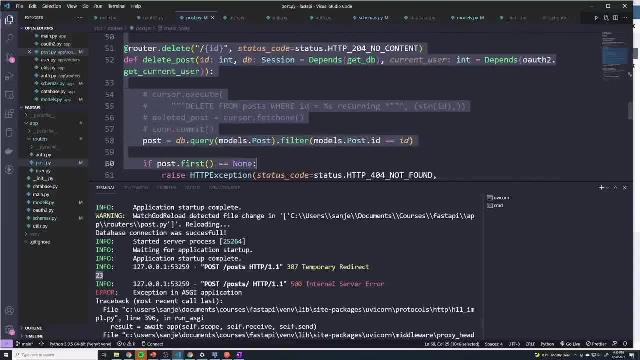 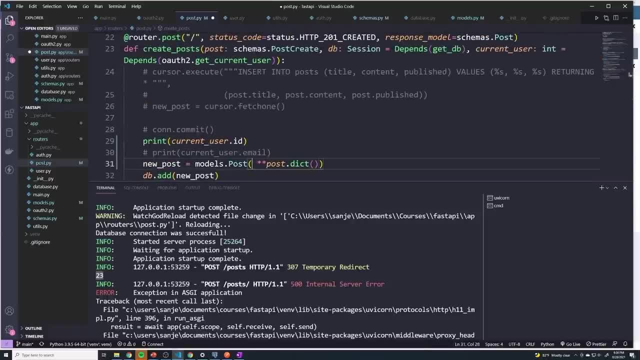 Right here where we reference models that post, And what we're doing is we're just spreading- whoops, we're just spreading out the schema that we got from the body, And so to actually add the ID property, it's very easy. All we have to do is just say owner underscore. 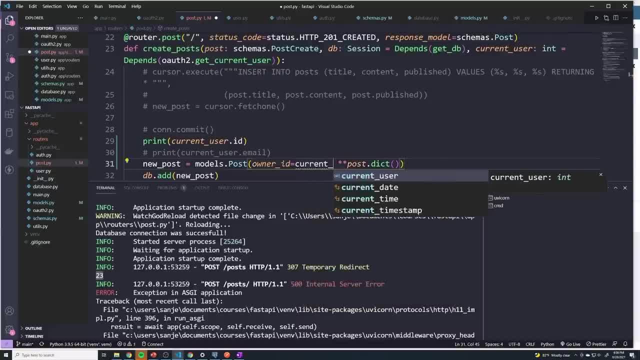 ID is going to be set to current underscore user dot ID. So we're just grabbing that from the get current user function, just like we did right here, And I think we probably need a comma there. Here we go, And that should be all that we have to do. So let's, I'm going to remove this. 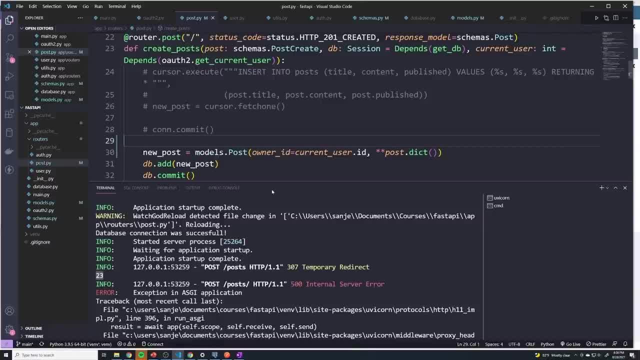 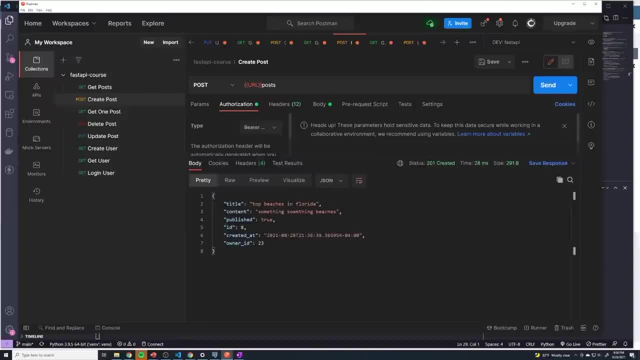 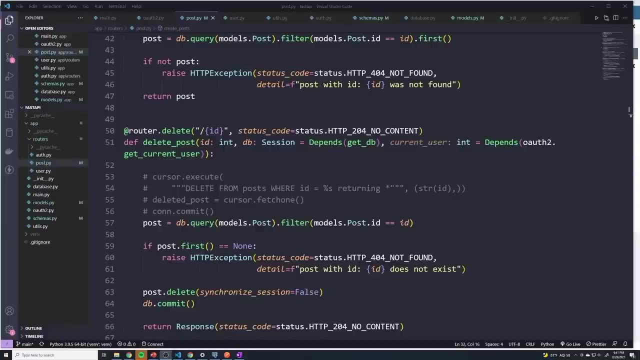 code And let's test this out now. So if I do create post, look at that and no errors. you can see that the owner ID was automatically set to the ID of my user, which is 23.. Currently in our application we do have authentication set up for delete post and update post. However, 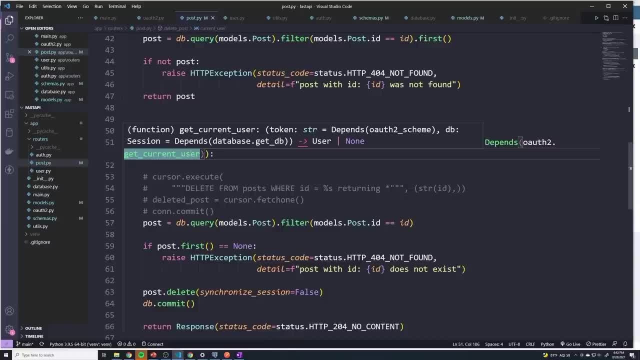 there's no check to make sure that a user is not set to the current user, So we're going to do that. And then we're going to do a little bit of a test here, So we're going to do. a user is only deleting his own posts Right now. if you're logged in, you can delete anyone's posts. 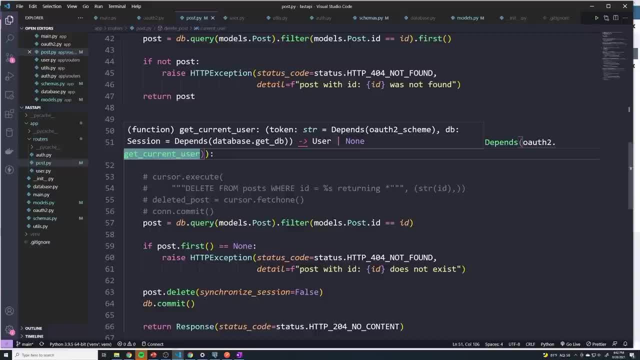 And no application works like that. You should only be able to delete your own post. No user should be able to come in and delete one of my posts. That doesn't make sense. So let's implement the logic for setting up a quick little just if statement. just to check: hey, is the person that's. 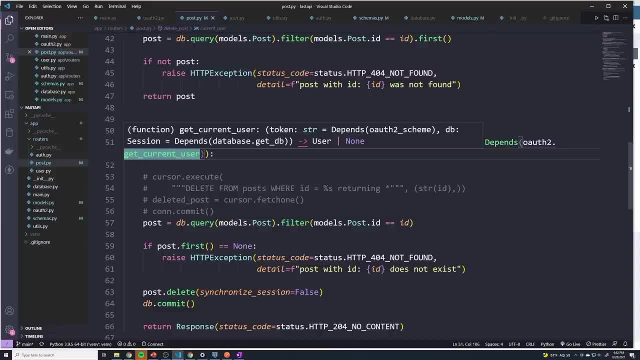 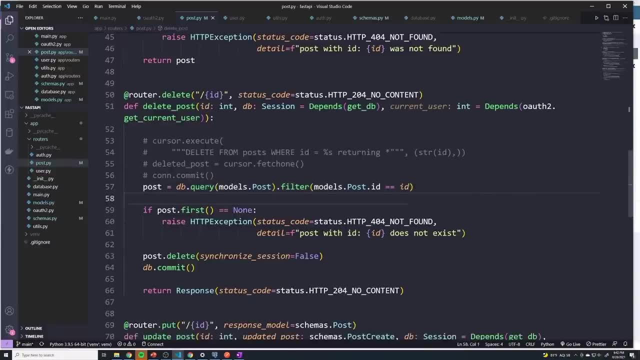 logged in trying to delete a post that he owns. If he doesn't, then we're going to return an error, And so right now, if you take a look at our delete post path operation function, we query the post that he's trying to delete And we check to see if there's no post. If 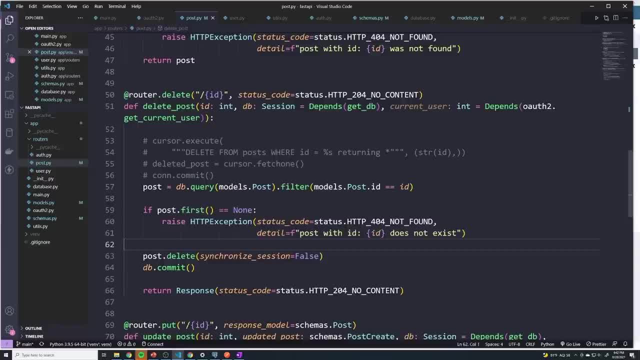 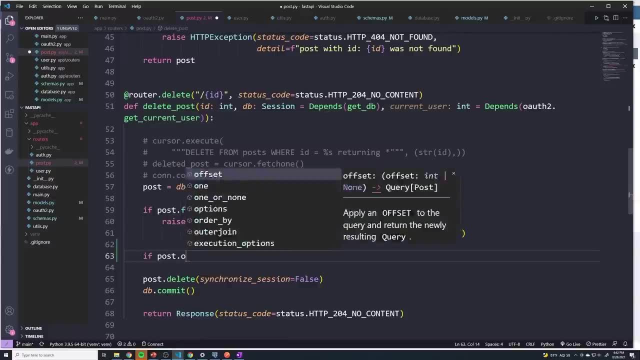 there's no post, then we send a 404. that's expected. But if we did find a post, the next check is just going to be another simple if statement And we're going to say: if post dot owner underscore ID does not equal, get current user dot ID. So these two things have to match. 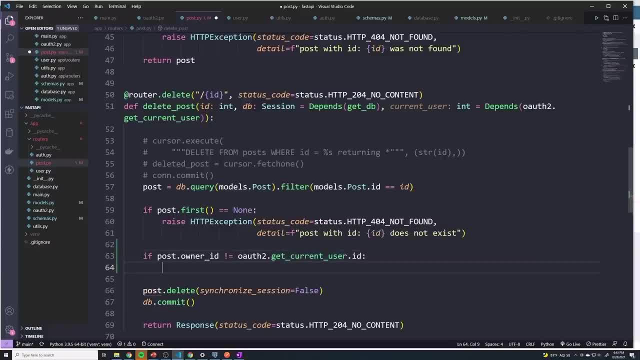 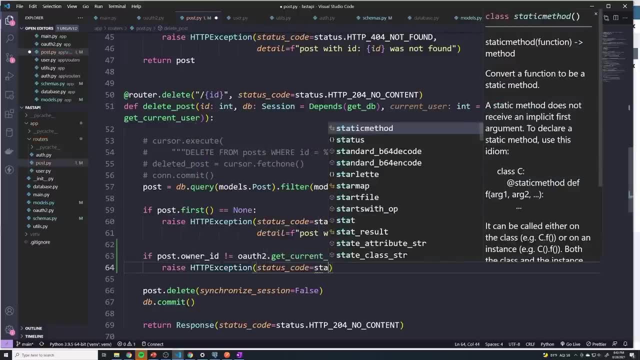 for the user to be able to delete it. If they don't match, then we're going to send another HTTP exception. So we'll say raise HTTP exception. Now the exception will set the status code to be a new one. So this one's going to be a 403.. So this means forbidden. That's the. that means it's. 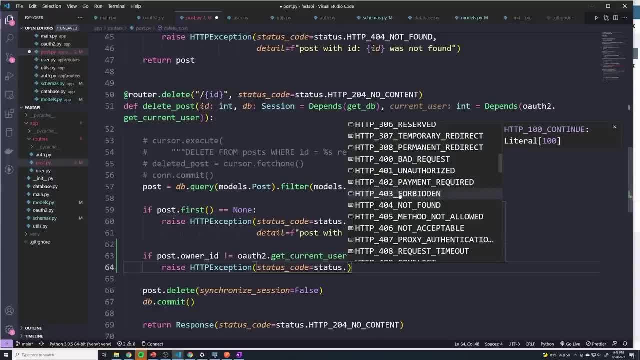 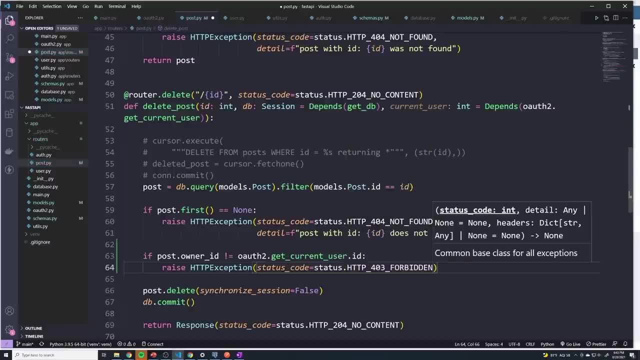 a resource that they specifically aren't able to access because on we could send a 401. But they are. I guess a 401 could also work, but I'm going to do 403.. I think that makes more sense, And then we can set the detail. And I'm just going to say: 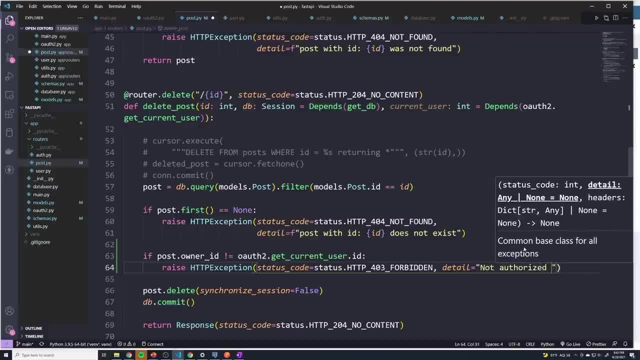 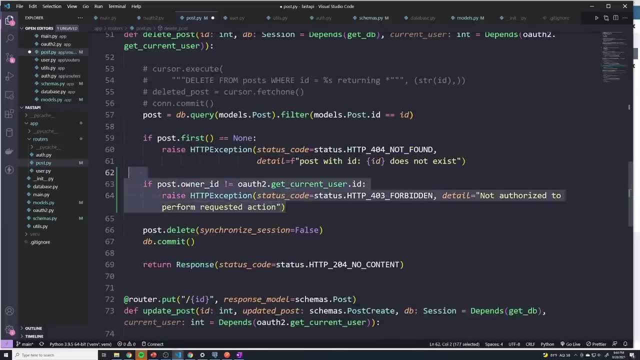 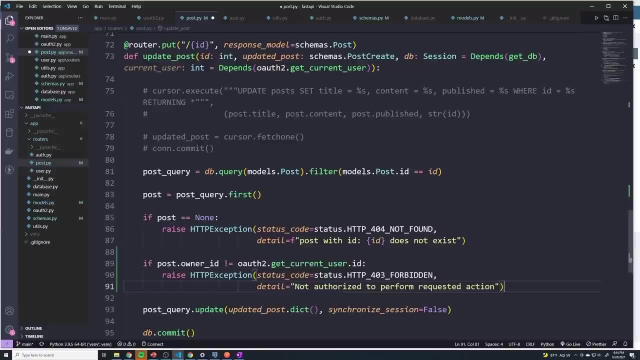 not going to do that, Not authorized to perform requested action. And this exact same check can be used for updating posts as well, because it's the same exact logic And I'll just do that right here, right under the same check. So same logic, right? First thing we're gonna do is we're 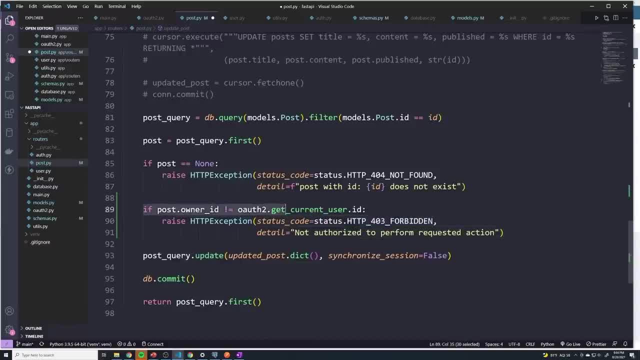 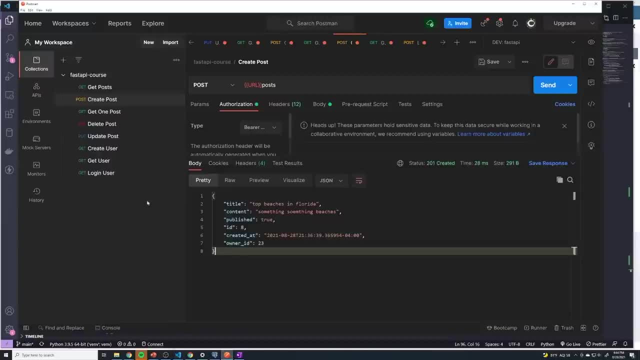 gonna check to see if that post exists And the next thing we're gonna do is we're going to make sure that the owner of the post is whoever the user is logged in as Now. let's test this out. So right now, if I do a get posts, you can see that the owner. okay, so we've got a post created by both. 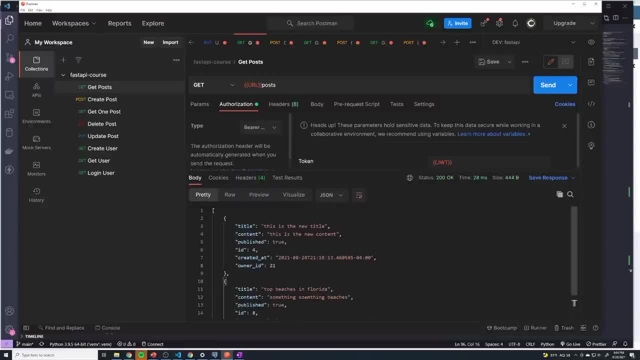 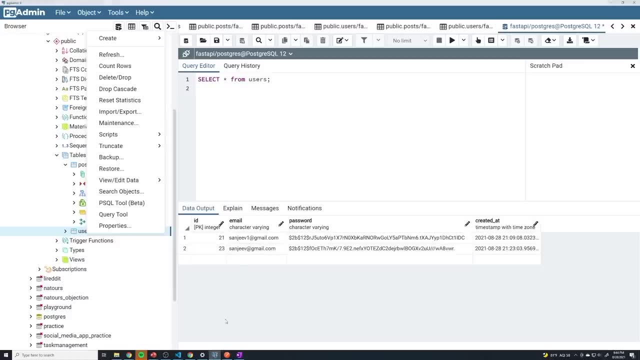 owners And I'm currently logged in, as. I actually can't remember who I'm logged in as, But we can see that I used Sanjeev at Gmail and that's going to be user 23.. And what I'm going to do is go back to. 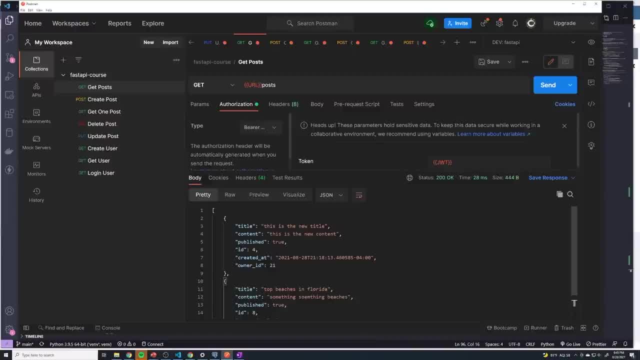 get posts And I'm going to try to delete the post with an ID of four, because that's the owner ID of 21.. And keep in mind, right now I'm logged in as user 23.. So let's try this. we're going to delete post with an idea for okay. 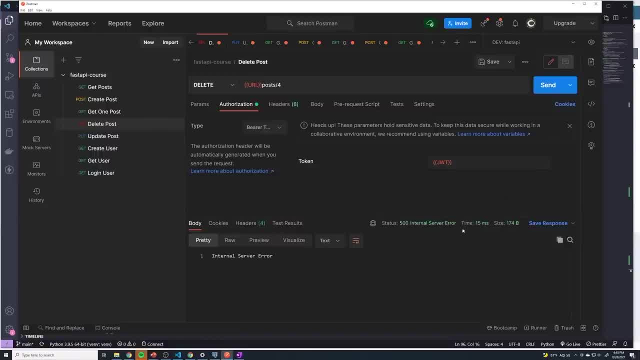 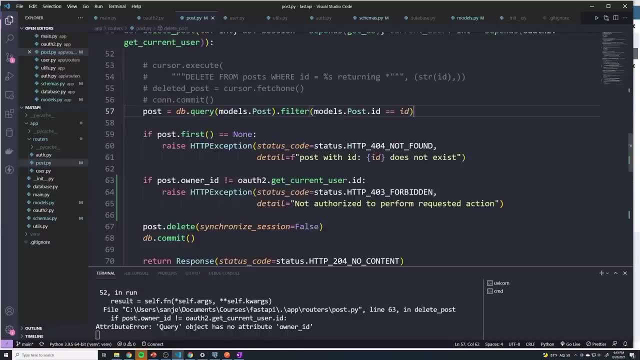 it's already set there, So we should get an error in this case And looks like I got a server error. That's a problem And I already see the issue. And right now, post is actually not the post itself, it's the query And to actually get a post I have to do post dot. 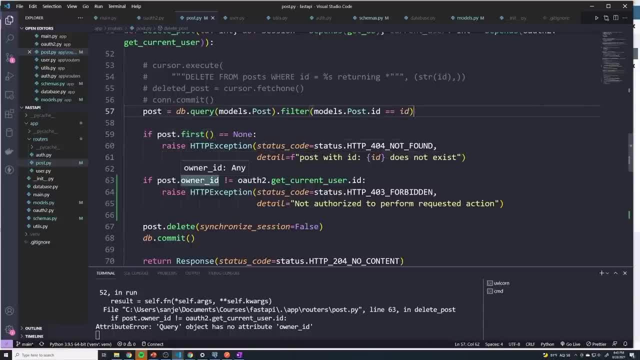 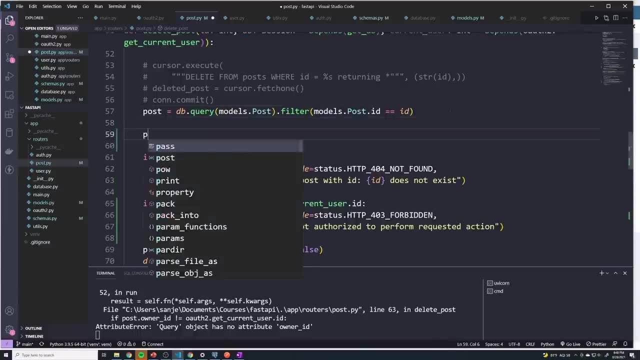 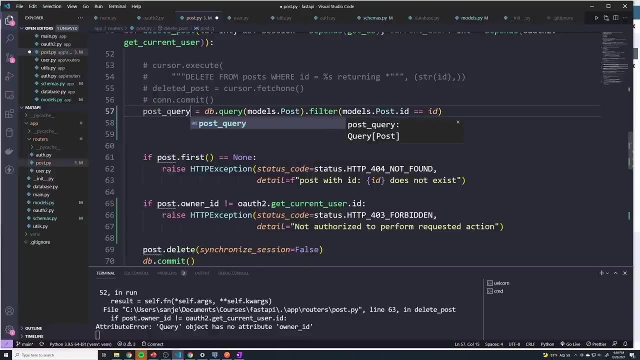 first one. So what I'm going to do actually is I could change this to post dot first and then grab the owner ID, but I'm going to actually perform the query right here. I'll say post Actually. I'll change this to post underscore query. I'm going to make a few changes actually. 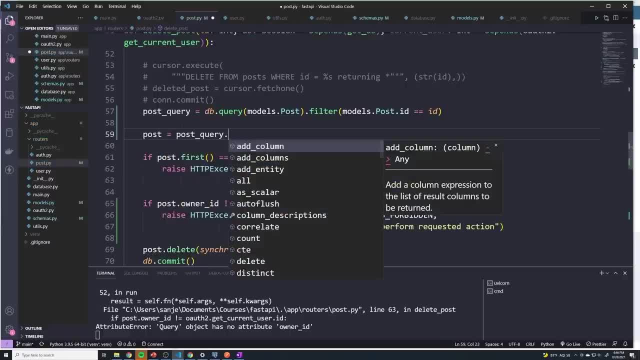 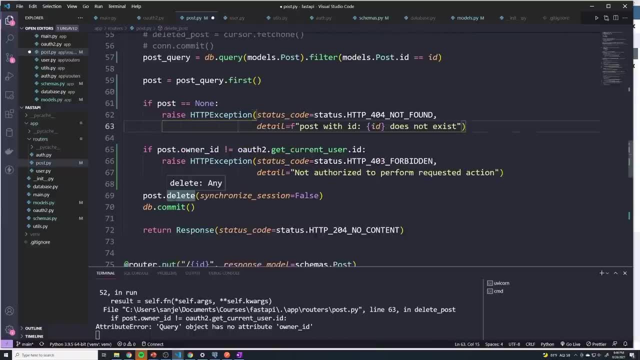 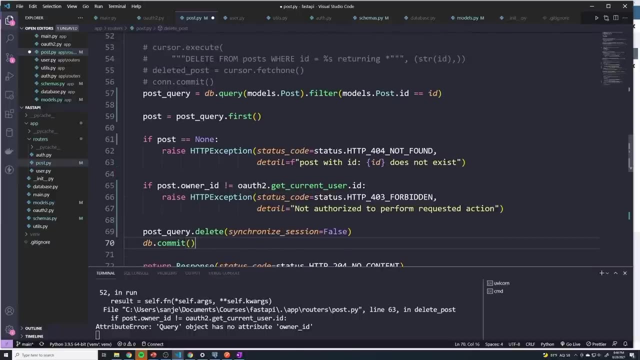 And I'm going to set this to be post. equals post. underscore query dot first, And then I'm going to set this to be post And this is going to be set to query. All right, and just to kind of quickly recap, we define the query here. we'll then find this post. 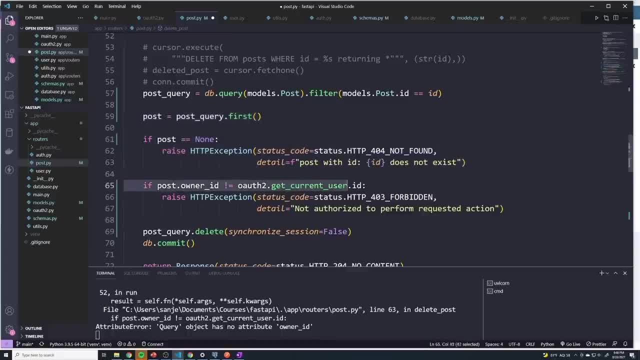 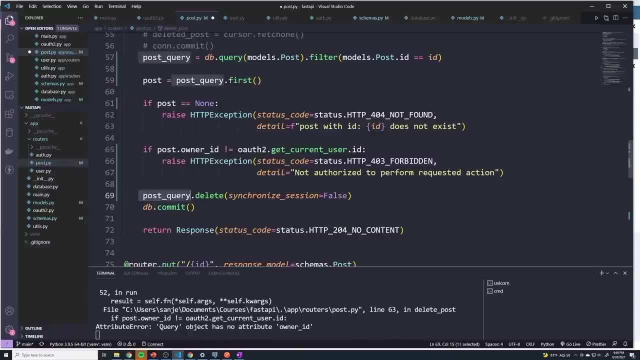 we'll check to see if it's not there, And then we'll check to see if the owner is, if the user who's logged in actually owns this post, And then we're going to grab the original query And then we're just going to append a delete, that we delete it, That's all, And let's just make sure the update. 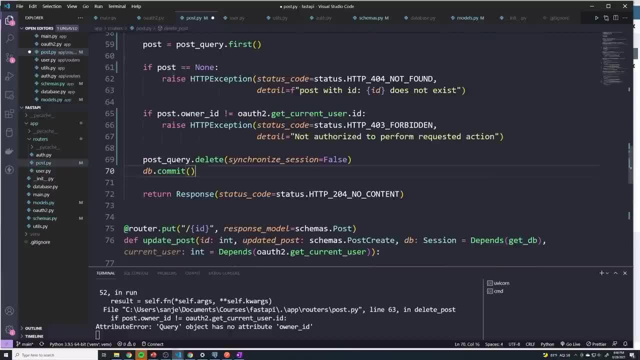 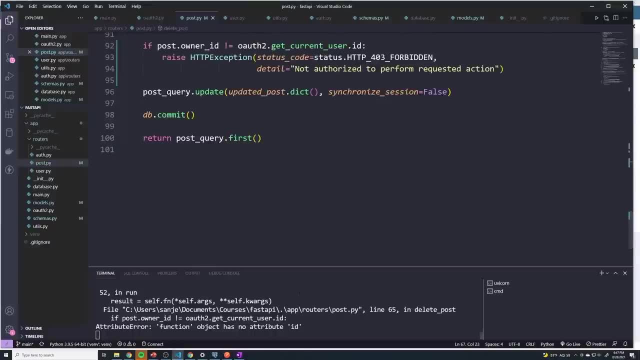 is set up the same way And it looks like the update one was already working that way, So it should be good to go now- Hopefully there's no errors- And let's try this. And once again we got an error. 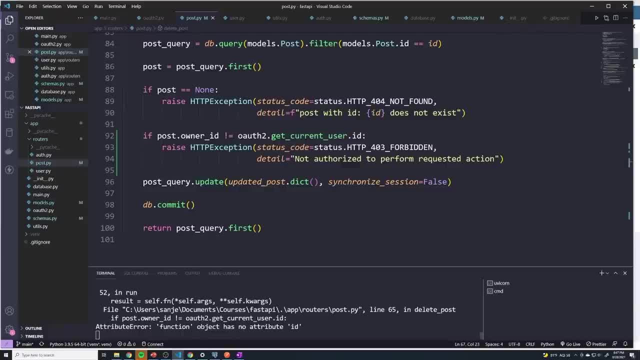 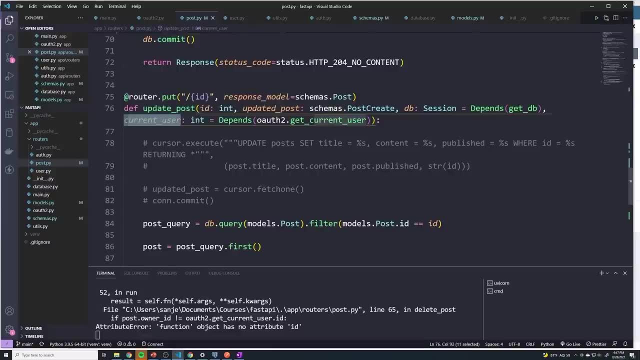 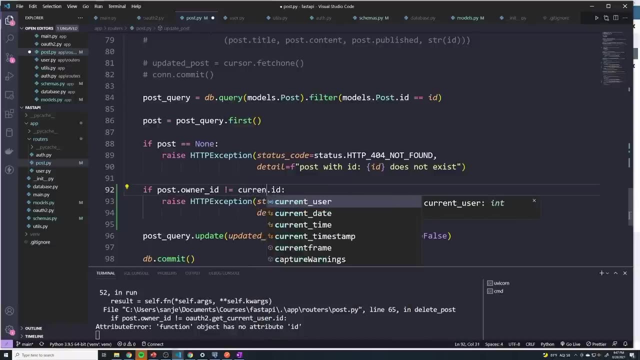 And it looks like function object has no attribute ID And I realized my mistake Again. first of all, this is getting stored as current user, not get current user, So we need to change this to be current user. I'm not sure why I did it like that. Seems pretty goofy. 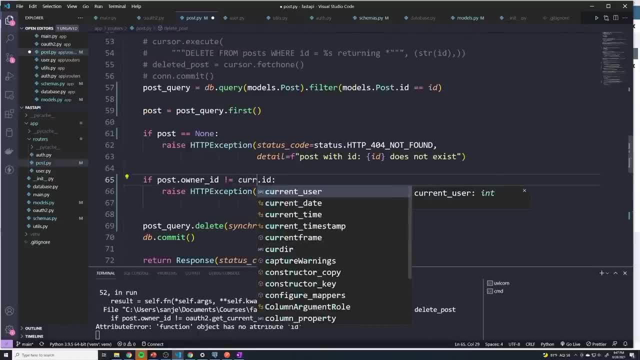 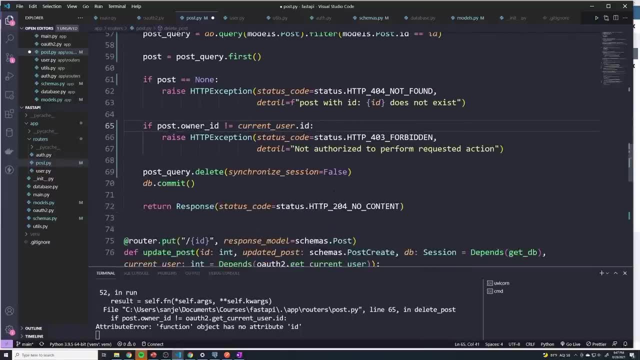 And then this also should be set to be post, And then this should be current user Right, because we're calling that function and we're storing the result in current user. So we want to reference the variable. I'm not sure if that was. 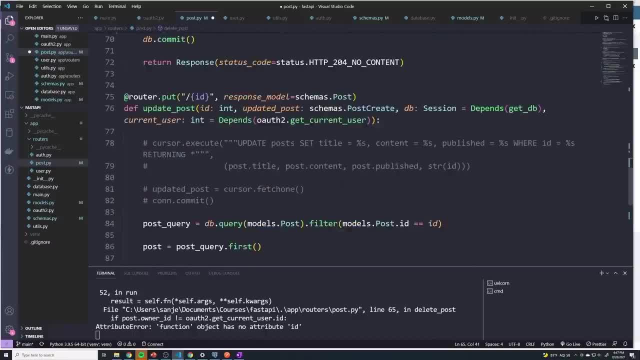 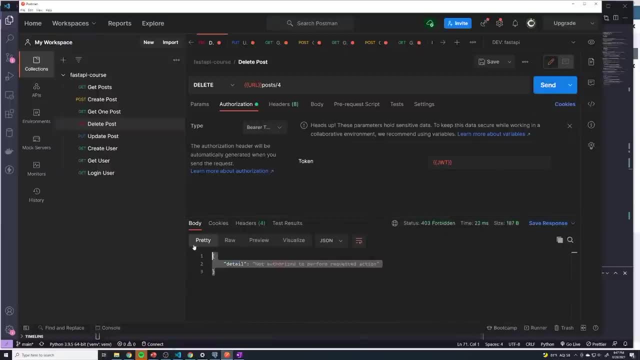 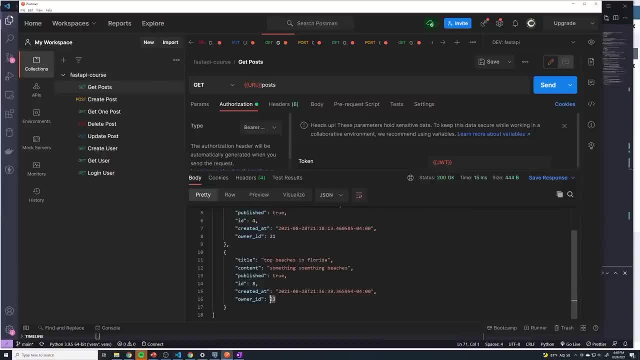 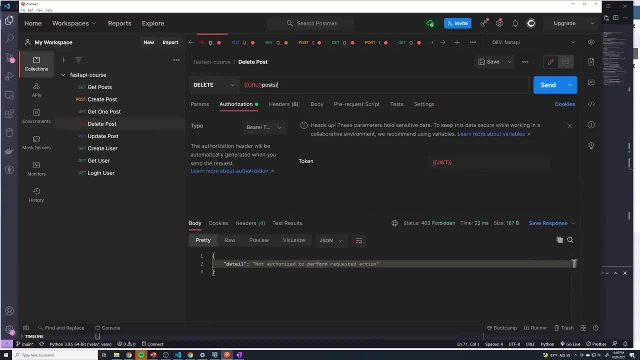 logged in as. So let's try to delete post with a value of eight Send and we get a 204.. So that means it's successfully deleted. we'll do get posts, just to verify, And we can see that we get those. just the one post now. So that seems to be working. I'm going to go back in. Actually, let me. 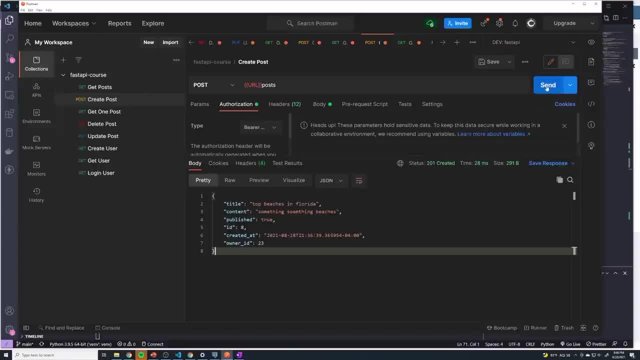 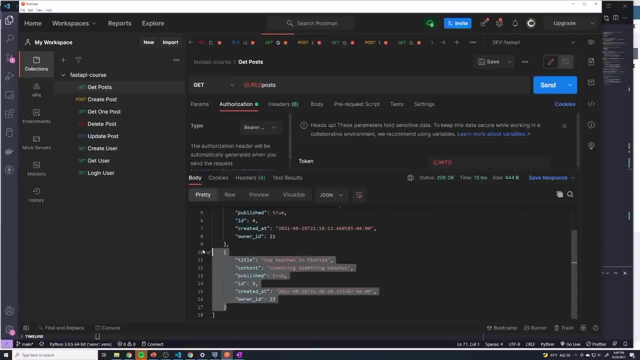 create a post real quick because I no longer have a post, Alright. so we have, we created a new post, And so you can see that this is my post right here And I'm going to just update it. So let's go. 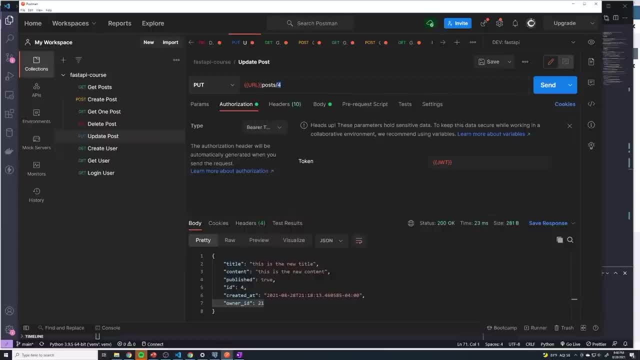 to the update one. First of all, I'm going to try to update a post that I don't own, So we're going to try to update the post with an ID of four. we should get a not authorized, And then let's grab. 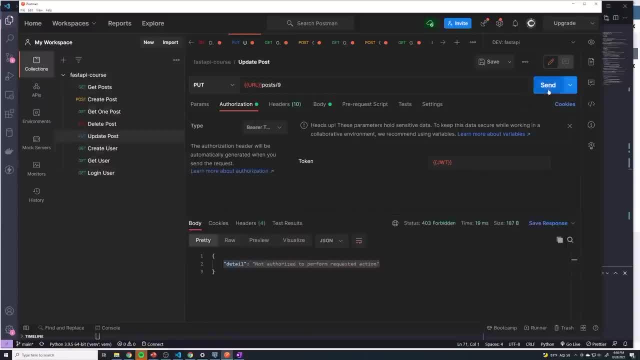 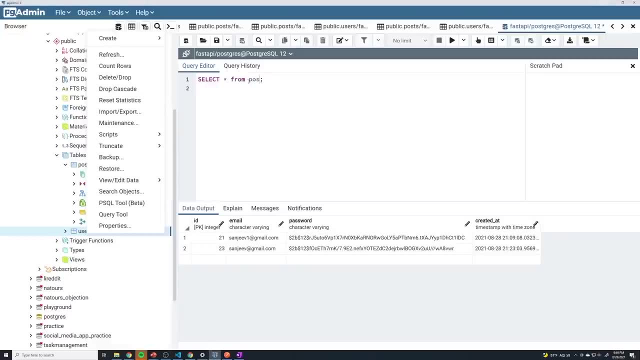 the ID of the post that we do want to change, which is nine. Let's hit send And it looks like it updated a little bit. Let's check our database always, So we'll say select star from posts And the post with the nine got the update And then we're going to go back to the post And then we're 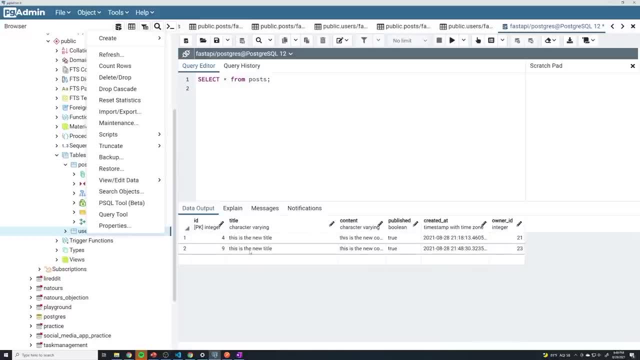 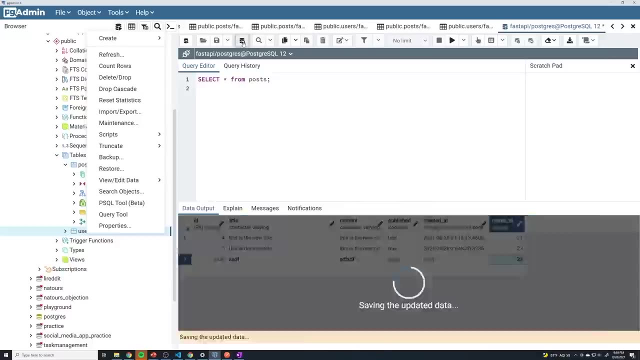 going to say: Oh wait, wait a minute. it looks like it may have updated both of them. Only one way to find out if that's actually what's happening: I'm just going to create a quick new post. I'm just going to set the ID to be 23.. Alright, and I'm going to update post with nine. 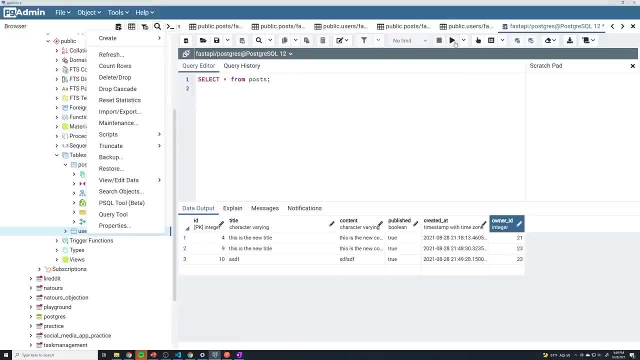 with an ID of nine. Okay, and then let's refresh this. Okay, so post with an ID of 10 is still the same. So, okay, it wasn't a bug. It looks like maybe I had changed this earlier, And I'm not exactly sure why I had when. 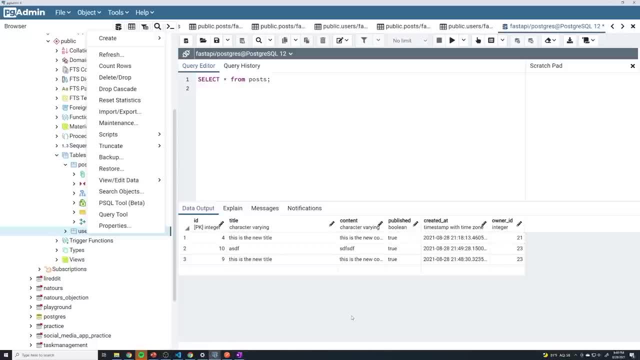 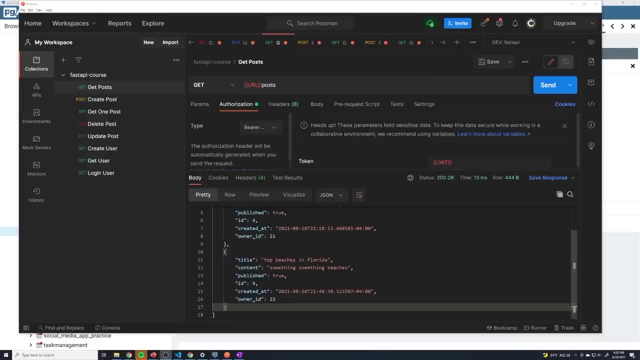 I updated this post, but that's okay, And so I think that's going to wrap up this video. We've handled the update and delete so that we can only update and delete our own posts. All right, before we proceed any further, I do want to talk about one last thing. 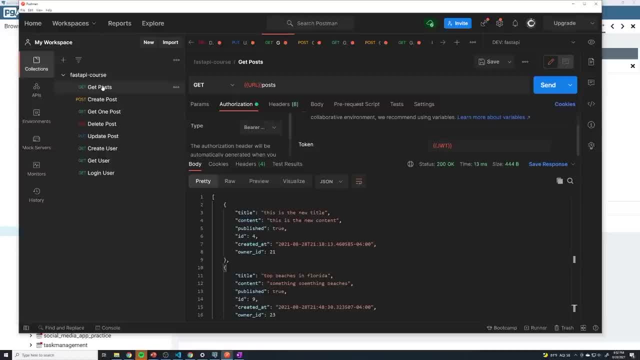 And that is that when we do get posts, which is an authenticated route, so it requires you to be logged in to retrieve the posts. If I try to retrieve the post, you'll see I get posts from the user. Now this may or may not be the result that you want, right, It's going to depend on what. 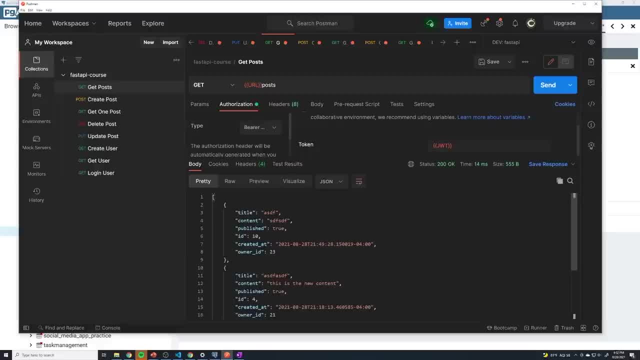 your application is going to work. look like. You know, if this is like a, you know, like a note taking app or something where all of your posts and things like that are all private, then you wouldn't want to return everyone else's posts, you'd only want to return the user, the user. 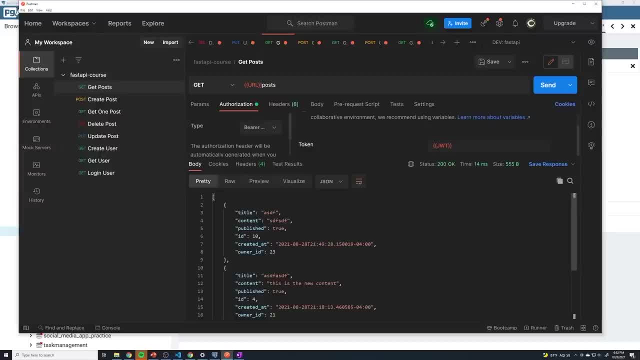 specific post. However, if this is some kind of social media app, right then obviously your posts are public. So when you do get posts, you'd want to return everyone's posts, And so it really just comes down to how you want your app to function. I'm going to show you, guys, what you would need to. 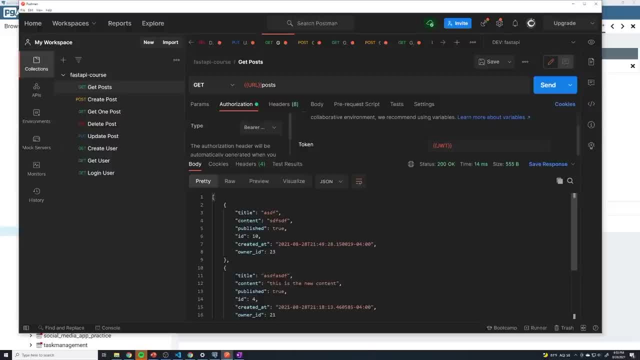 change if you wanted, to make it so that you return to your only your own posts, But after afterwards we're going to actually delete those changes because I want to leave my app like this. this is kind of how I wanted it to work, more like a social media app, But I do want to make sure that 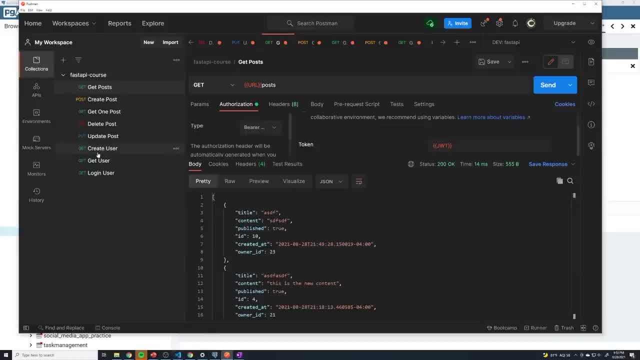 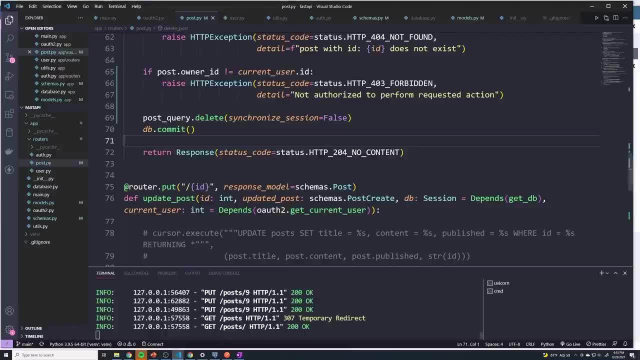 you guys understood how to make this change, And the same thing would go for get one post. we want to make sure that only the user that created a post can retrieve that specific post, And so if we go back to our path operation for getting all posts, 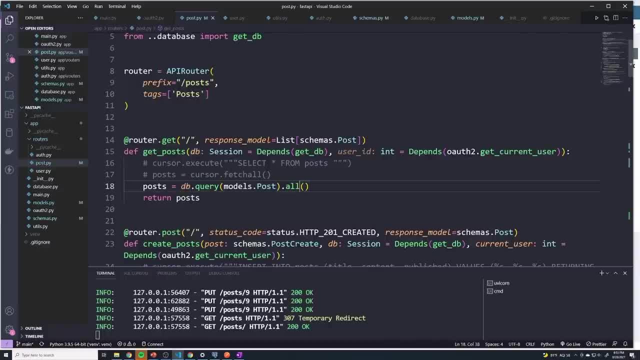 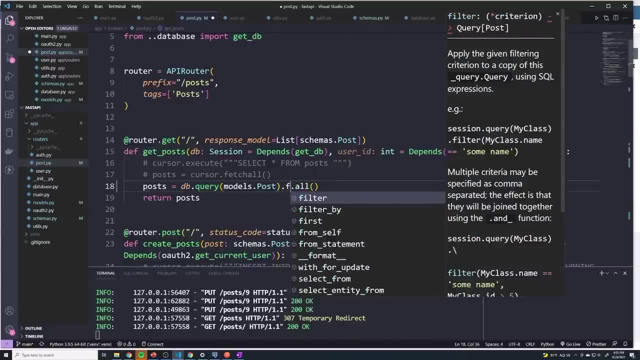 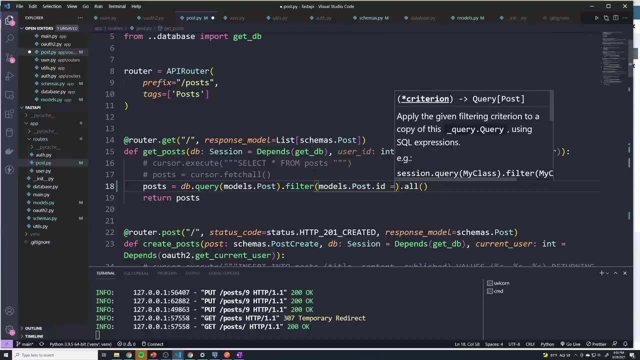 you can see that we just do a db dot query dot all, And so if you only want to return the post for a specific user that's logged in, it's very simple. all we have to do is do a filter And here we'll say models, dot, post, dot, ID, equals, equals. And then we just get the current users ID. 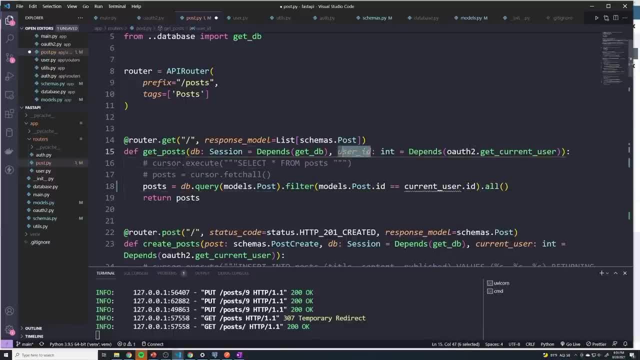 And it looks like I still left this as user ID, So this should actually be updated to be current underscore user. And if you notice the, you can see that the type is set to int, even though it's actually returning an entire user object. I found that this, whatever type you put, 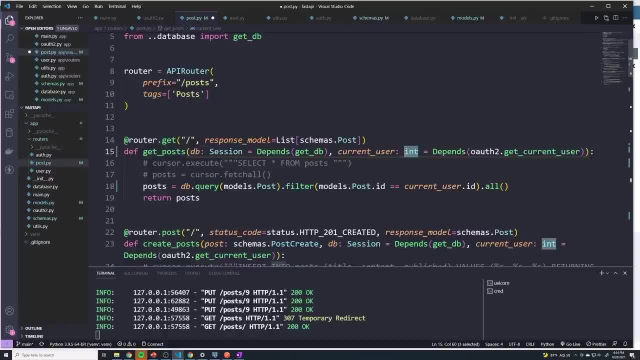 here doesn't actually impact the code. So put whatever you want. you can put in a you know some sort of dictionary that actually correctly matches it, But you could just leave it as well. So I'm just gonna leave it like that. It doesn't break any logic. And then at this point, 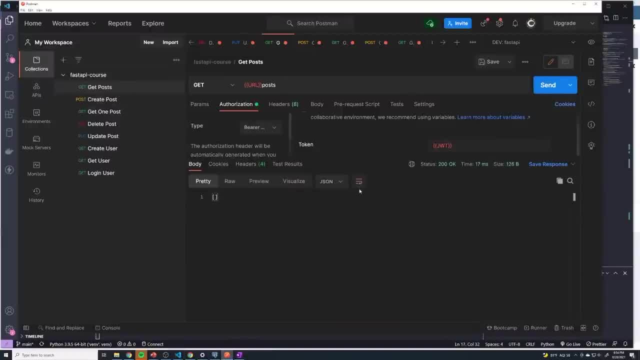 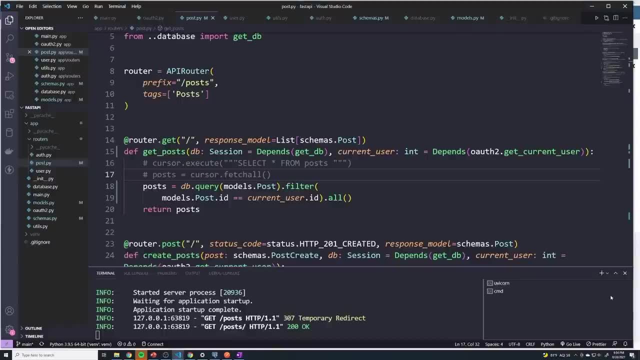 I believe I'm still logged in as user 23.. If I try to retrieve all posts, looks like I got nothing And that could be a little bit of a problem. So let's see what we broke And the easiest way to kind of troubleshoot. this is what I'm going to do- is I'm actually 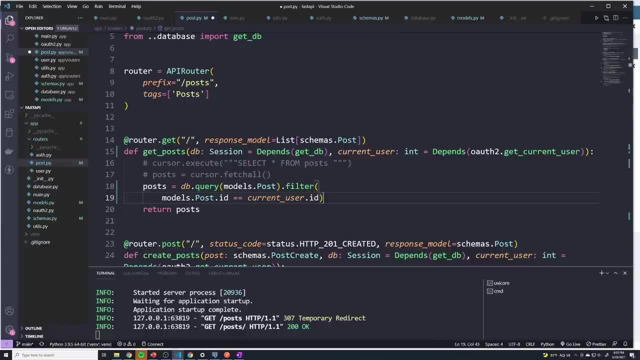 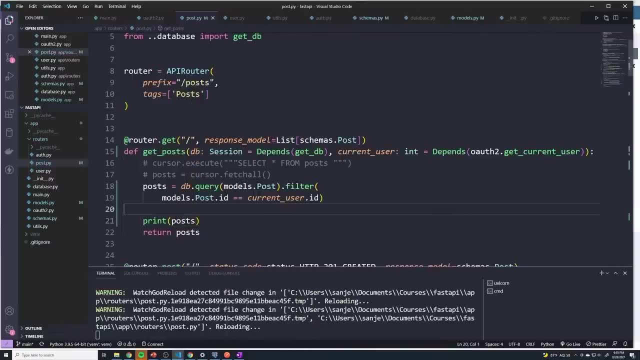 going to remove the dot all, So that's going to return the query. it just won't actually run the query And I'm just going to print the query. Let's see what that looks like. Sometimes it helps to see the raw SQL. Let's hit send Alright, we should get an internal server. 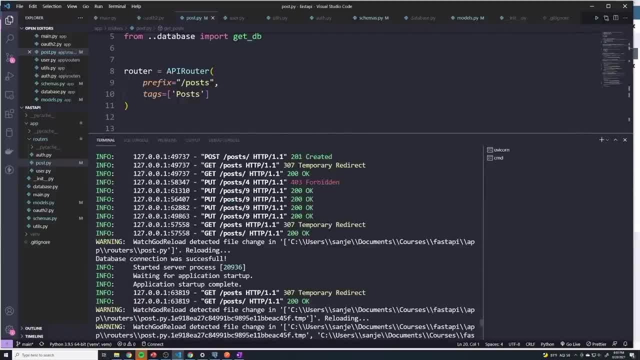 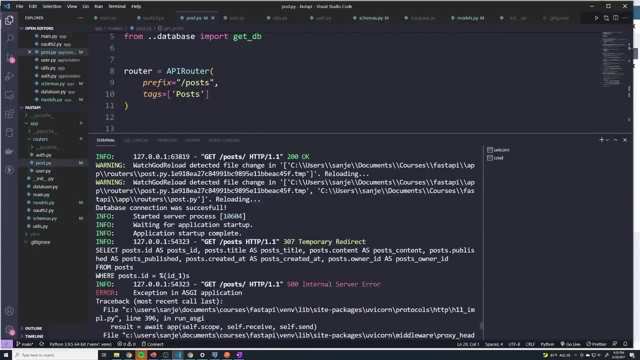 error. that's to be expected, But I just want to see my print statement, Alright, so let's see our print statement. So, select: we're getting all the columns that's expected from posts where posts ID equals this value, So that looks like it's perfect, Well. 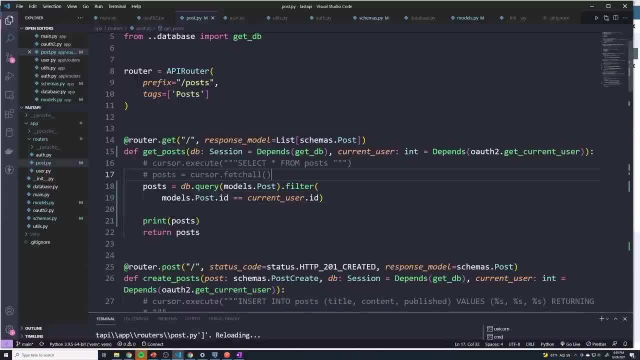 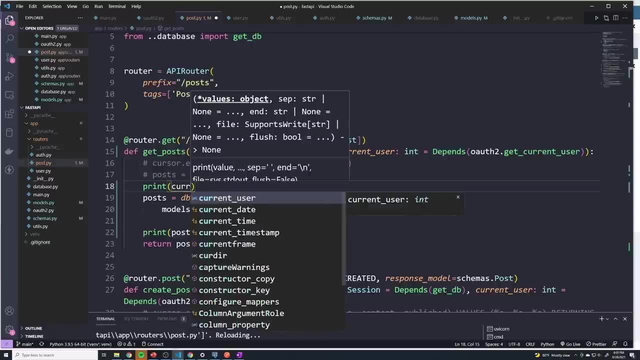 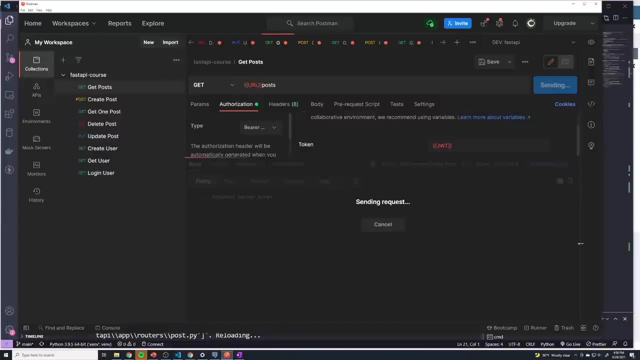 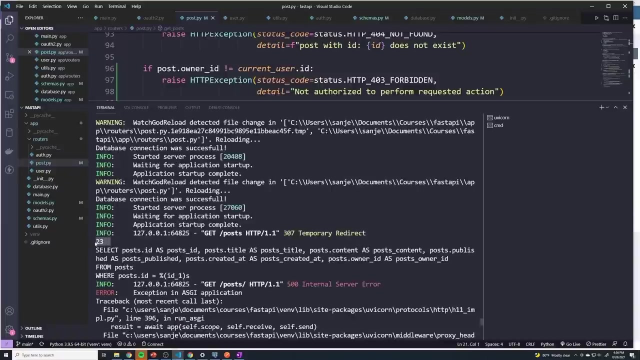 let's just quickly see, Before we move any further, what exactly is my user ID, and we'll just check our database. Okay, and we'll run this again, And then we're going to check, Right, so 23.. And then, if we go to our database, 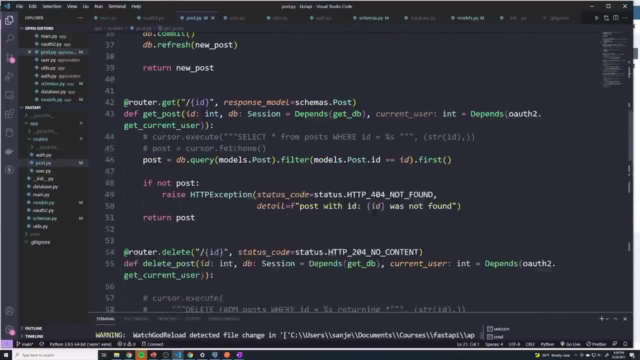 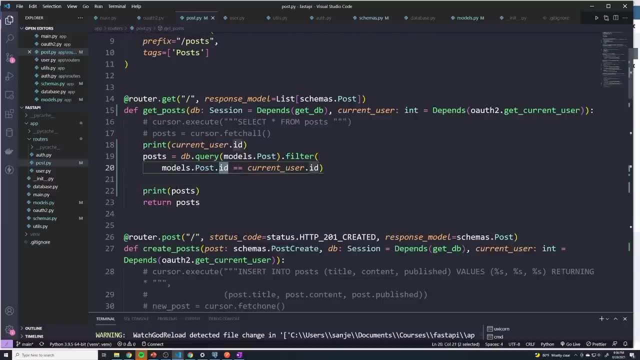 and I realized the exact mistake that I made, and this is a stupid mistake, Right? this is: this is looking for a post with an ID with this specific ID. we don't want the the ID of the post, we want the owner ID. So we'll do. owner. underscore ID equals current user ID. 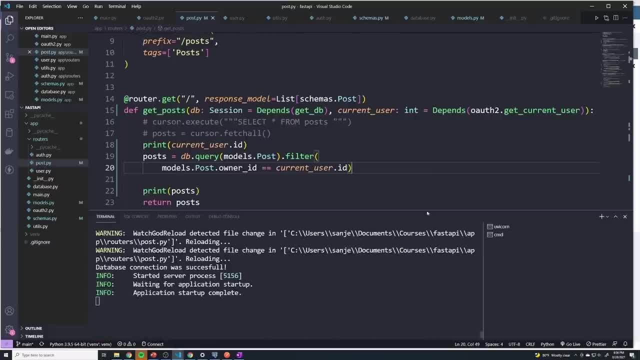 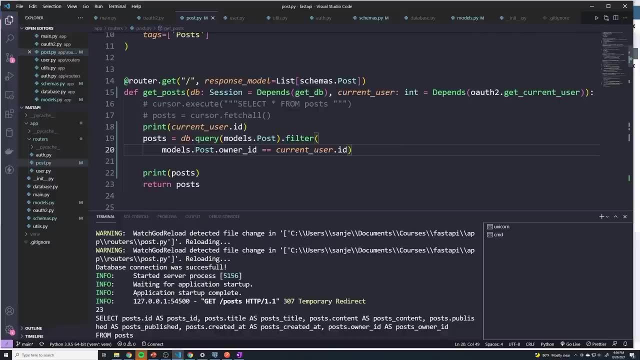 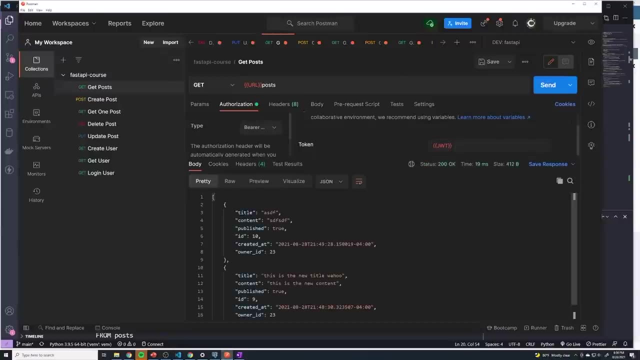 And then we'll just test this out. Alright, let's test this out now. Once again an error, but I just realized I forgot to update this to be dot all, And then we'll try this again. And now we get all the posts with an ID of 23.. 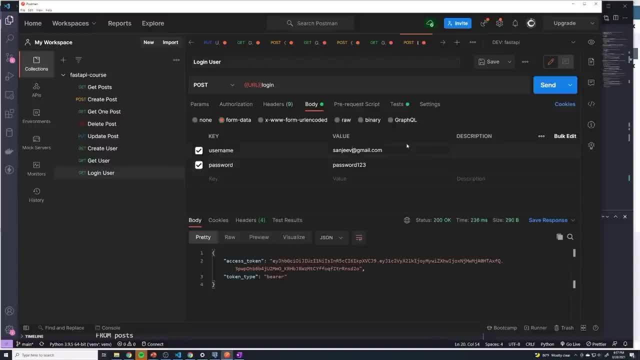 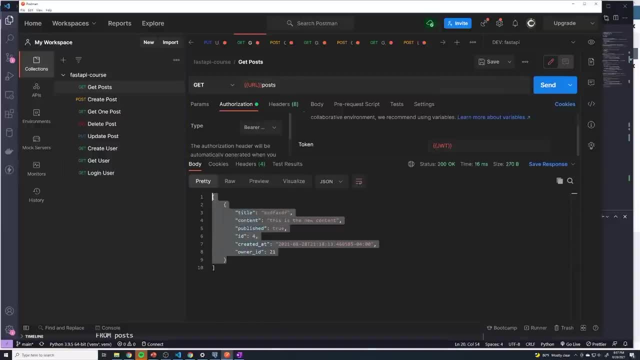 If I log in as a different user- let's say this is Sanjeev one- I'll log in. that should update the token. So now, if I do a get all posts, it should return all posts with an ID of 21.. And so that's, that's how that works. And then, if you want to see how that looks, 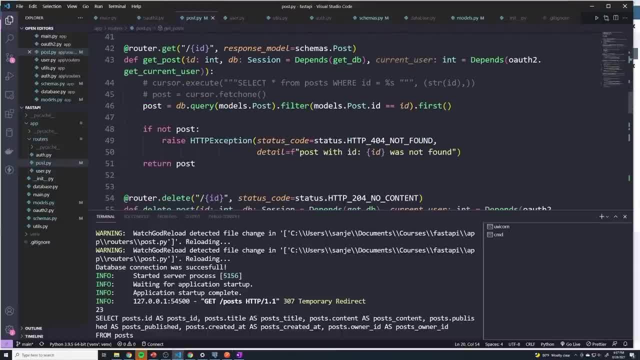 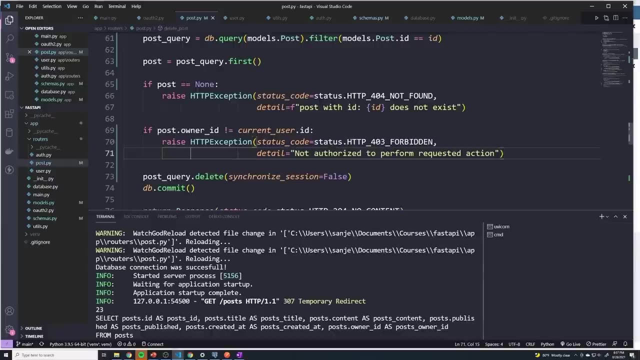 like for retrieving an individual post, we'll go to get underscore post And to actually handle this logic it's going to be the same thing as a delete. So you can just copy what we did for the delete one And here I can just say: post that owner. 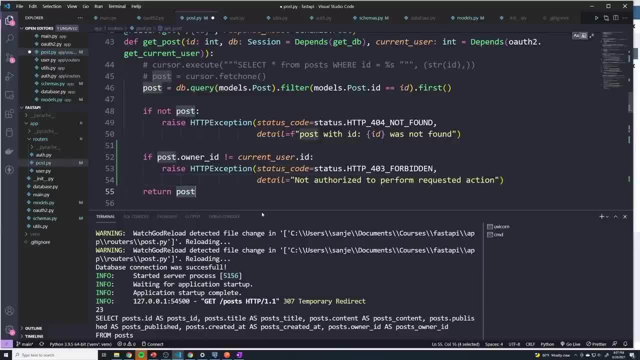 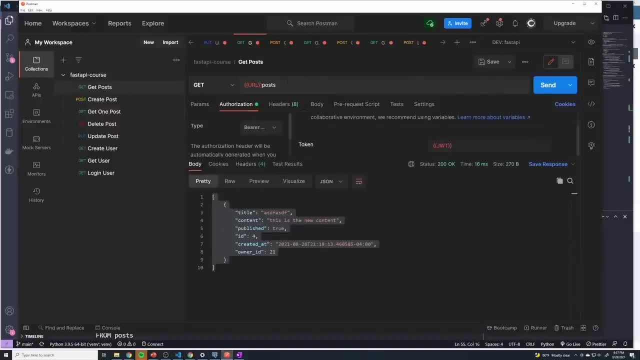 And this should do the same exact thing. So now, if I do get one post, well, first of all, let's take a look at all of our posts. I'm going to do it in our database. So I'm logged in as user 21.. 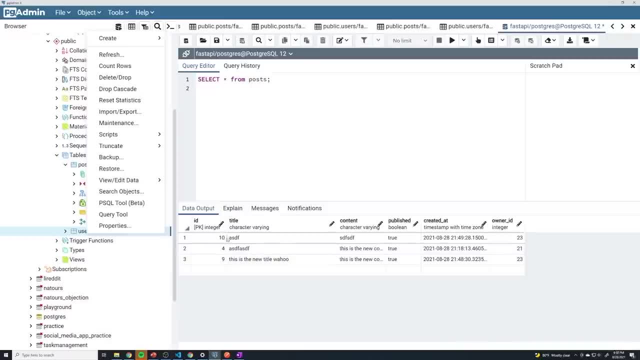 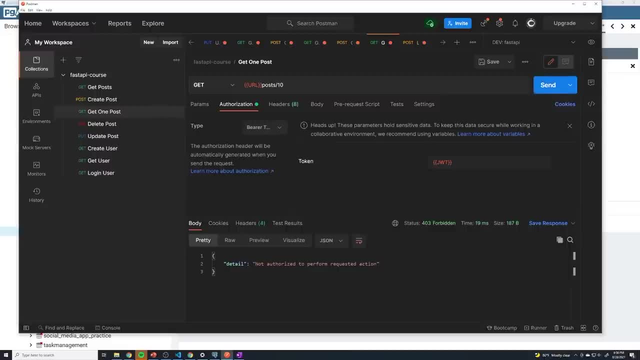 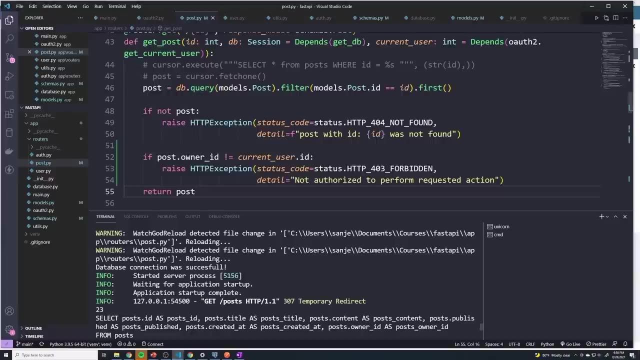 So I should be able to access a post with four, but I can't access a post with an ID of 10.. So let's try 10.. Am I able to access him Not authorized? Let's try ID of four And I can get that one. So that's how that works. But, like I said, I don't want my application to 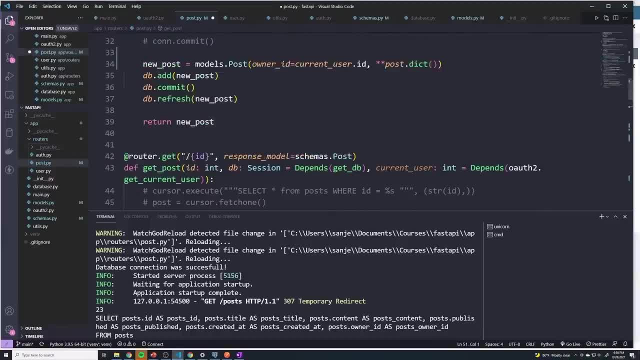 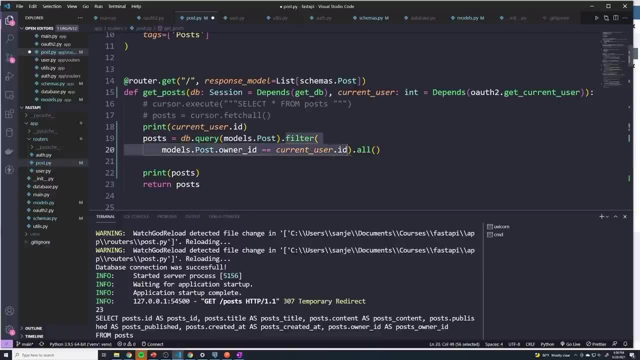 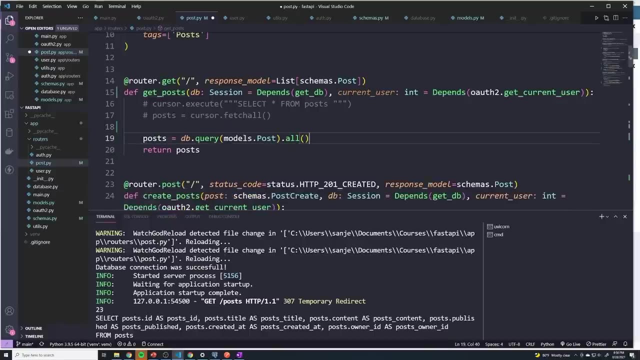 work like that. So I'm going to remove that functionality, I'm going to make all posts essentially public And then we're going to remove this filter And I'll remove this print statement and this print statement, just to clean things up a bit And let's just double check that. 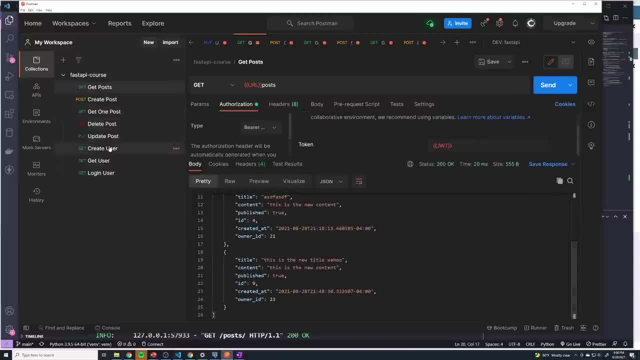 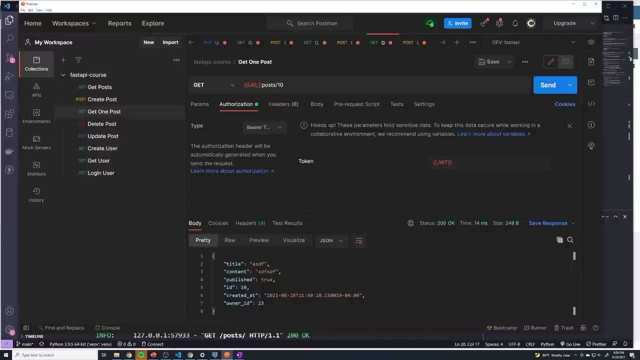 we didn't break anything once again. So let's get all posts, we get all posts, Let's get an individual post, Regardless of who owns it, And that's all fine and dandy. now. Now, just kind of thinking ahead of what our- you know- front end would look like. 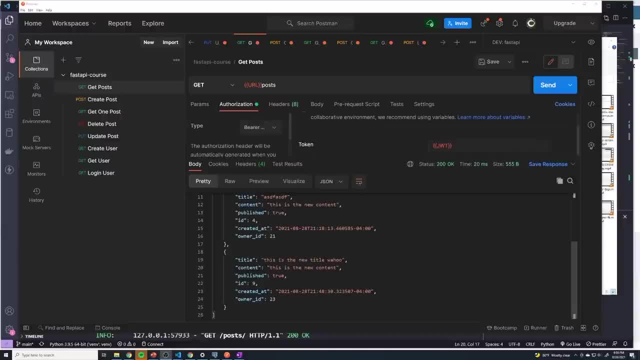 even though we're not going to build it. Taking a look at any social media type application, you know when we retrieve the posts, we usually want to embed the users ID. So we want to know who actually created the specific post. we wouldn't just put the owner ID because no, no user. 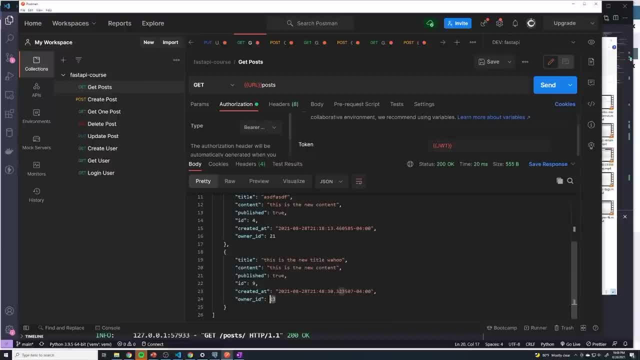 your users understand that id. they want to see what is your- you know- twitter handle, what is your email? whoever created that, we want to see their user id. so it looks like for all of the posts that we retrieve, we would have to then send a second query to retrieve. you know, hey, what is. 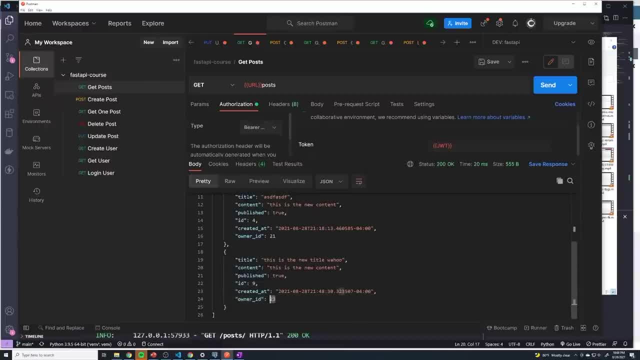 the information for user uh with an id of 23, and then, once we get that, we would then have to kind of combine all that data so that we can figure out what post uh it belongs to what user and what is their specific username. now with sql alchemy we can kind of set up. 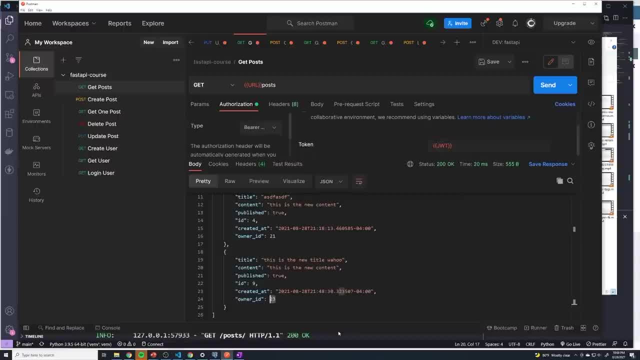 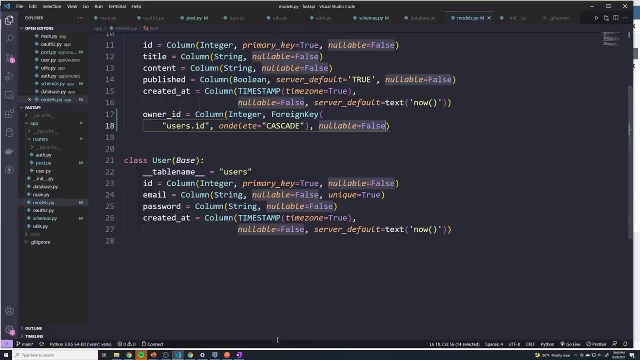 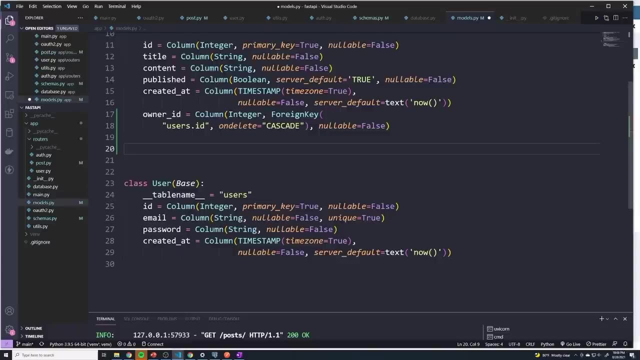 set it up so that it automatically does this for us, and so, if we actually go to our models, what i'm going to do is i'm going to set up a relationship, and so this relationship isn't a foreign key. it does nothing in the database whatsoever, but what it does is it'll tell. 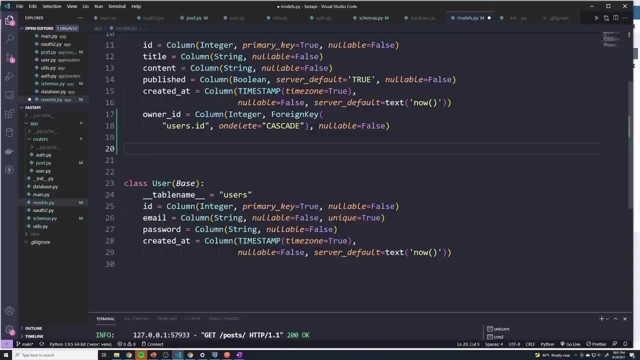 sql alchemy to automatically fetch some piece of information based off of the relationship. and so we're going to set up a relationship, and we're going to set up a relationship, and we're going to set up a relationship, and so here i could say we'll create a owner. 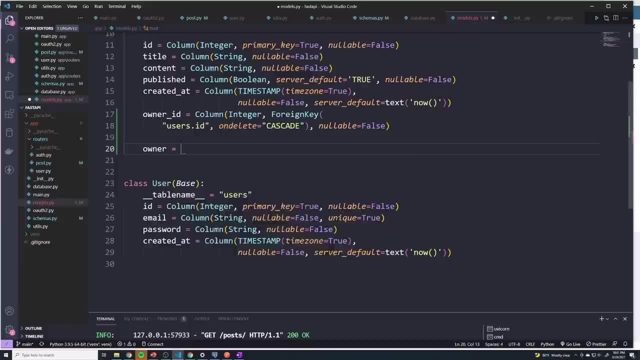 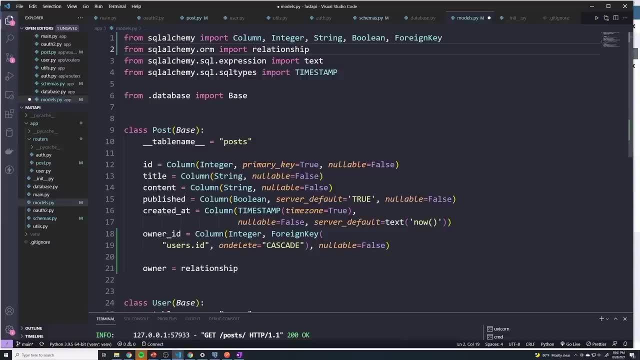 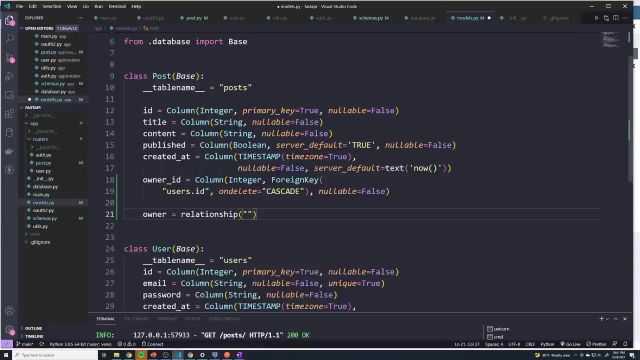 and i'm going to say: owner equals relationship and we probably have to import this. and so it did. so it imported relationship from sql alchemyorm and so if you haven't done that, go ahead and do that, and what we'll say is: this is going to return, uh, the class of another model. so here i want to return the user. 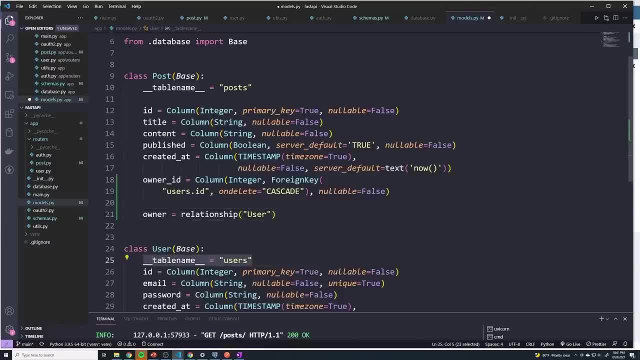 and this is going to be a capital u because i'm not referencing the table. i'm referencing the actual sql alchemy class. so what this is going to do for us automatically is that it's going to create another property for our post, so that when we retrieve a post, it's going to return a owner. 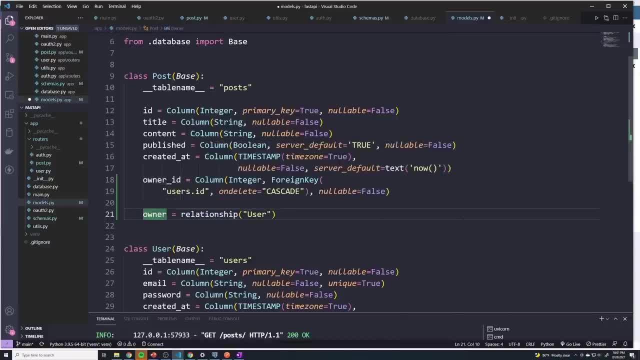 property and what it's going to do is it's going to figure out the relationship uh to user. so it's going to actually fetch the user based off of the owner id and return that for us and there's nothing else we have to do. it actually is that symbol. this is one of the great parts about sql. 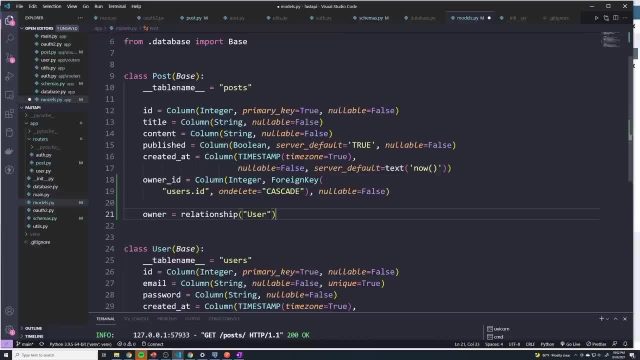 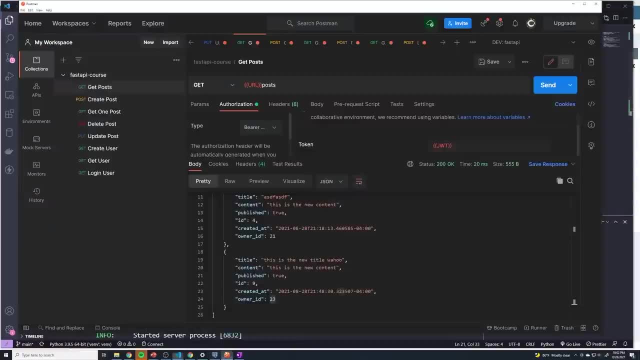 these relationships will automatically make it so that it fetches that data for us, so that we don't have to manually do it ourselves. so let's test this out, let's see if this actually works. i'm going to go back and i'm going to retrieve all posts and it looks like nothing's changed. we 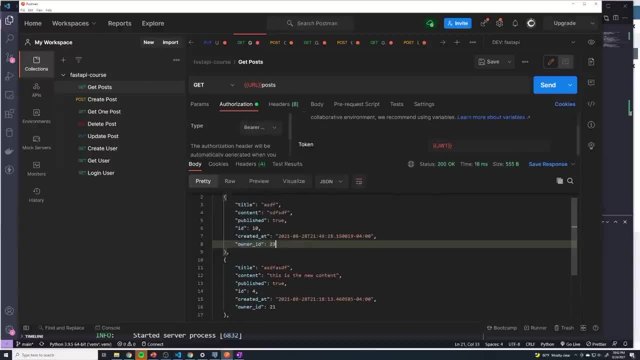 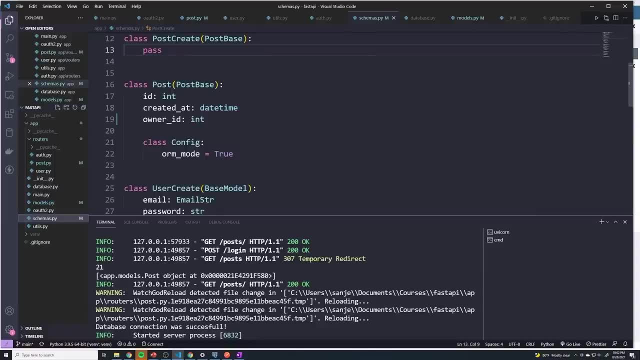 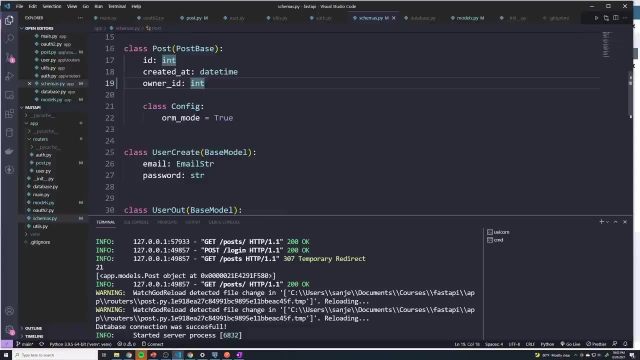 don't get any user information, we do, once again, just get the owner id. so what happened? well, you probably can guess. we need to update our schema, and so, if we go to our post, we're now going to return a user. and so here what we would do is we would just add another property. 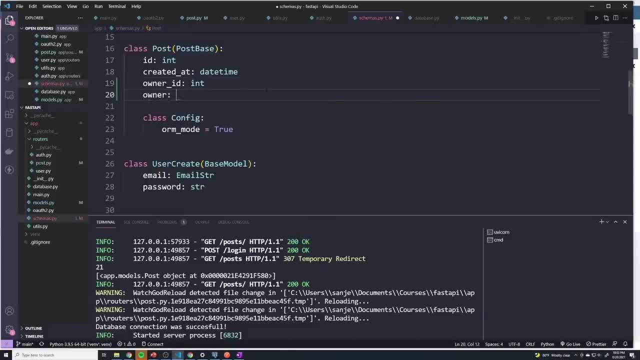 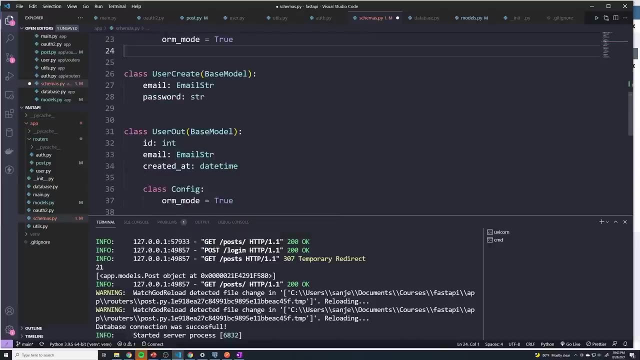 called owner, and then here it would. instead of returning an int or a string or anything like that, we can actually return a pydantic model. so i can say: i want you to return a user, what's a user? but it looks like we don't have a user class, we have user out and then we have user create. 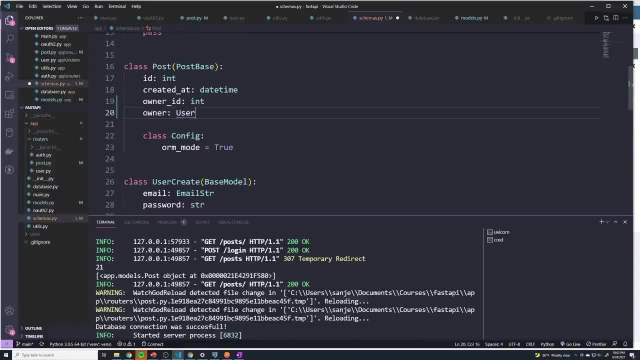 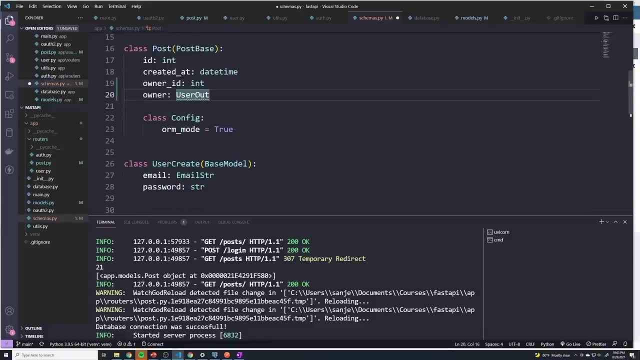 so which one do we actually want to return? um, probably user out, because that's what we're returning with the user. create is for creating a user, And you notice that we get an error actually here And that's because this user out hasn't been. 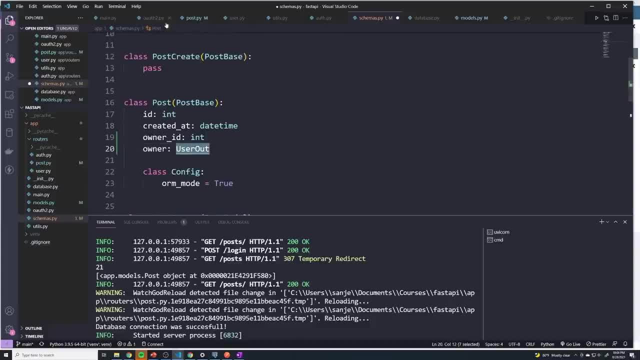 defined at this point in the code. So you have to read Python top down And so user out is actually defined all the way down here. So if you wanted this to work, we would have to move all of the user stuff up a level. So I'm going to cut this. images, put it right. 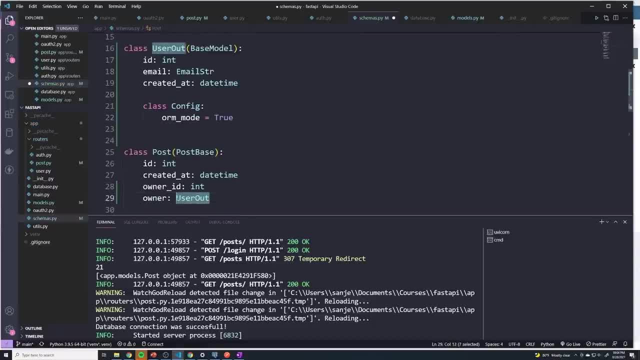 above post, And so this should remove the error, And so now it looks like it's good, And so, once again, all we did was we added a new property called owner, And this is going to return a pydantic model type called user out, And so that's all. this is returning now. 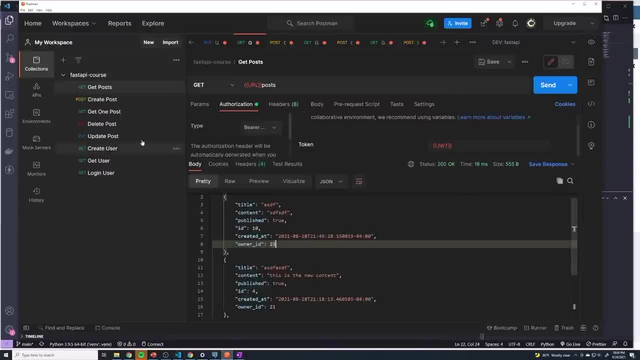 So let's see if this fixes our issue. And now I'm going to retrieve all posts. And so now take a look at this. it automatically fetched the owner. they got the ID, they got the email they got when their account was created at. we may not want that, But for now I think. 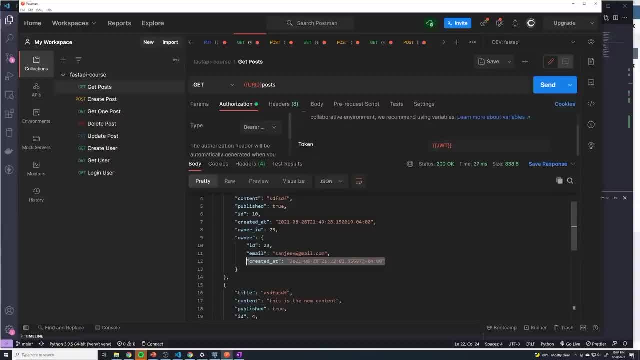 this makes sense. we could create another class to kind of narrow down the exact fields that we specifically wanted for this situation, But I think this is good enough. These are all the informations that I want actually returned. So this is perfect. It's going to. 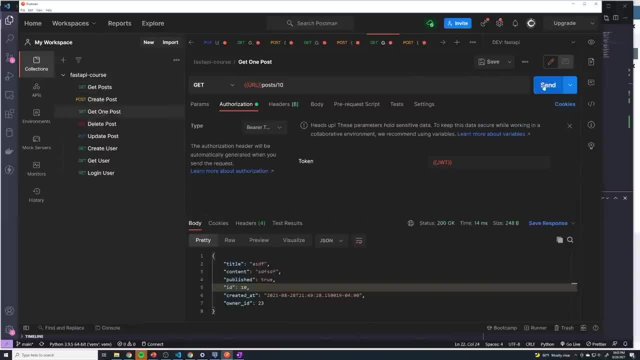 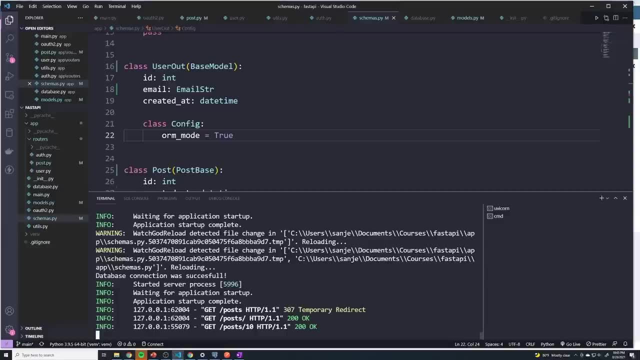 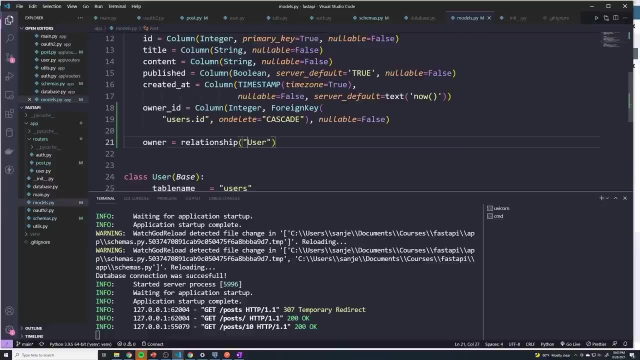 do this for every post, And if I try to get one post, it's also going to return. that's the pydantic, That specific owner, And so, in reality, to get this functionality by once again, all we had to do was just create this relationship, And so, once equal Alchemy understands the relationship, 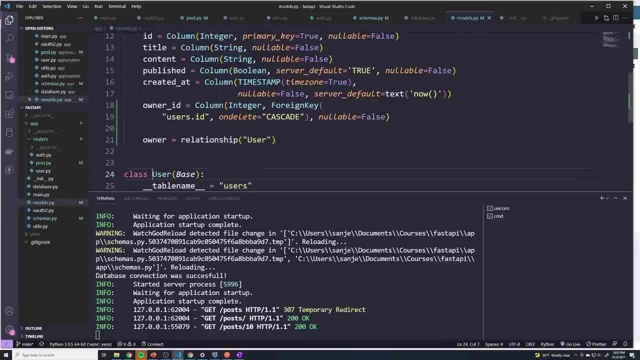 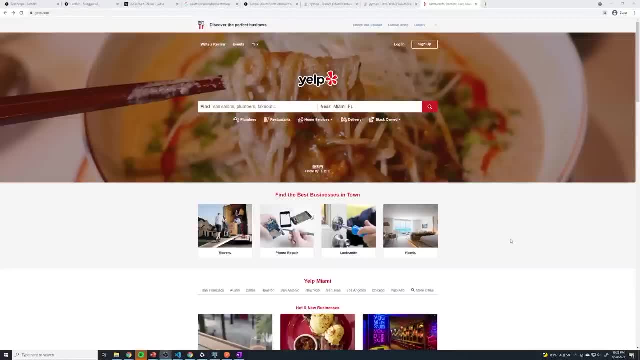 is going to fetch that piece of information for you from the user model. In this lesson we're going to take a look at query parameters, And if you've never worked with an API, you may not know what that is, But I guarantee you you have worked with them before And 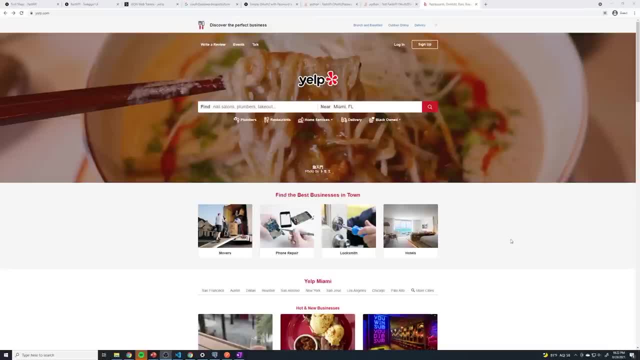 you have seen them, You just had no idea what they were. And so I'm on Yelpcom And I'm just going to go ahead and create a new API And here's where the data is required, And doing this for demonstration purposes. But I'm just going to do a quick search here. I've just 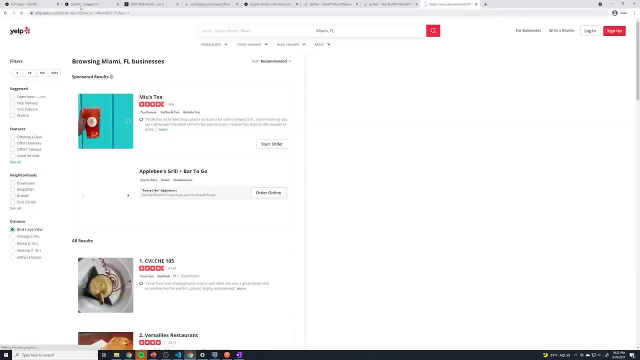 picked a random city. In this case it's Miami. we're going to search for that And I want you to take a look at the URL, And so our URL is: first of all, we have the domain name, which is kind of. 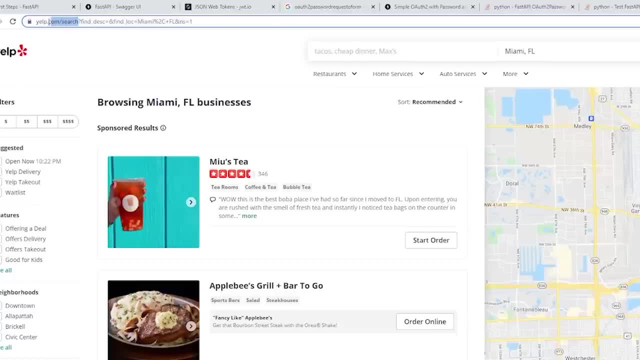 like the IP address, And then we have the specific endpoint that we want to reach. So this is the slash search endpoint. And so in their API they've set up, you know, some sort of endpoint that probably is allows you to search for restaurants. And then we have a question mark. 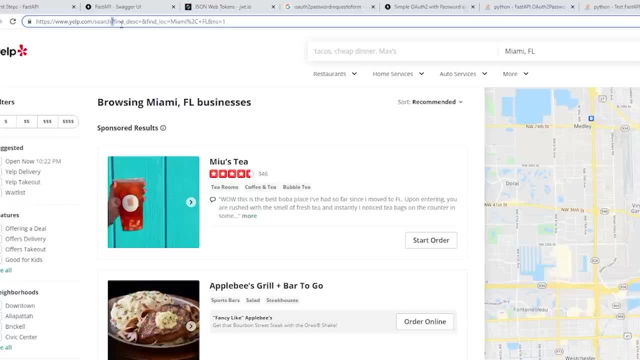 And I know you guys have seen this before, because pretty much any website you've ever, you know, used, you'll see that question mark whenever you're, you know, searching for things, And any results you get you'll see that in the URL, And so everything to the right of that is. 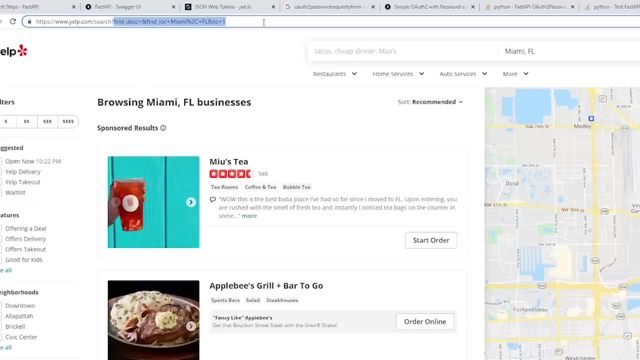 what's referred to as query parameters. So all of this is query parameters, And a query parameter is a optional key value pair that appears to the right of the question mark, And these query parameters allow us to kind of filter the results of a request. So you know if we're trying to. 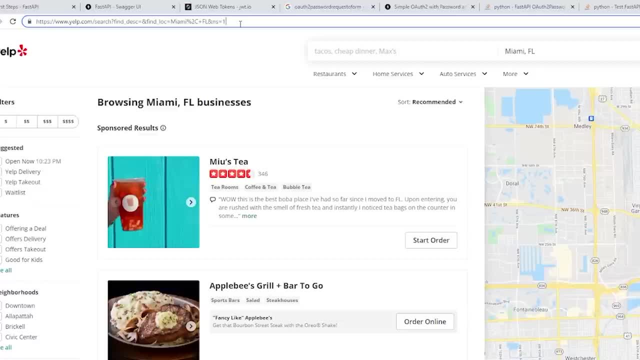 retrieve a request, we're going to have a query parameter And if we're trying to retrieve a post, maybe we don't want all posts. maybe we want to get posts that were created in the last two hours, maybe we want to get posts that you know, if it's a social media type app. 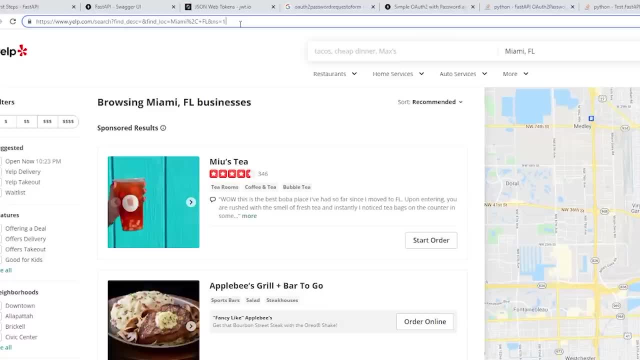 maybe we want to get posts that have received over 100 likes. right, these are all things that you would do using query parameters where you can say: hey, you could just pass in a key and a pair and you can say: I want to find posts, you know, that are less than two hours old, And so a lot of 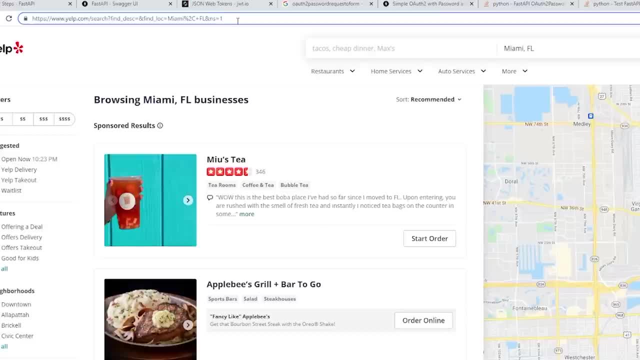 other operations that are necessary in an API, things like pagination. those are all going to be done with query parameters And so a lot of other operations that are necessary in an API parameters. And if you take a look at this one- since we searched for Miami, right, it looks like. 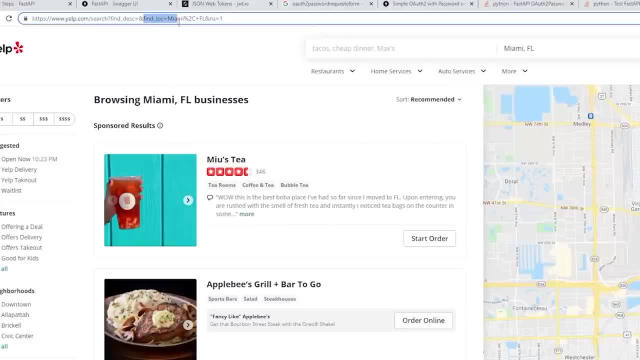 it passed a query parameter called find underscore loc, which probably means location, And then it says Miami, Florida, And so it's going to basically talk to the API and say: Hey, listen, I need you to get me all the restaurants And I want you to filter down based off of restaurants. 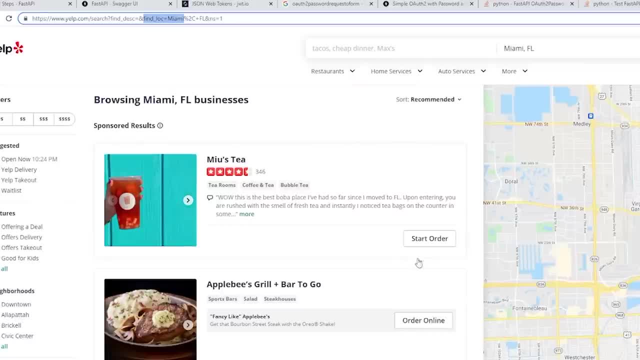 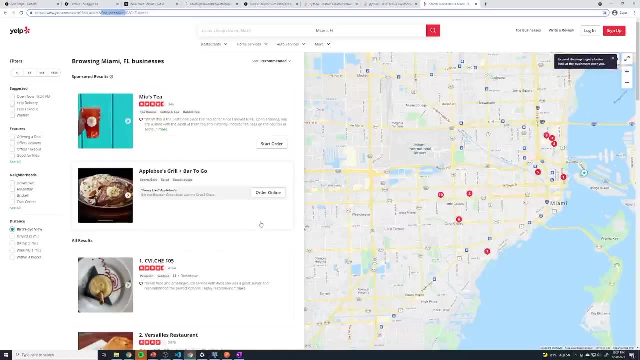 in Miami, And so that's kind of how query parameters work, And so for us it's. it's up to us to define what query parameters we want to allow and what we want them to do, And it's going to vary from app to app, But you'll see that most APIs have a lot of query parameters that are: 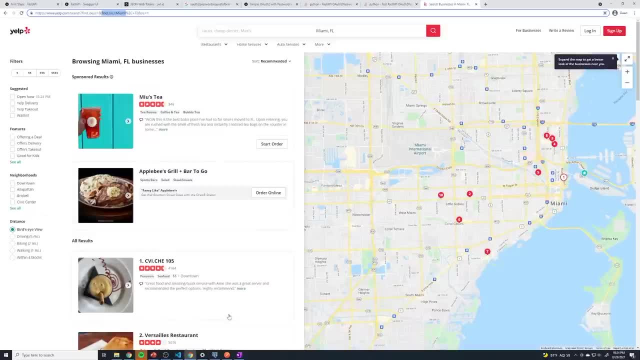 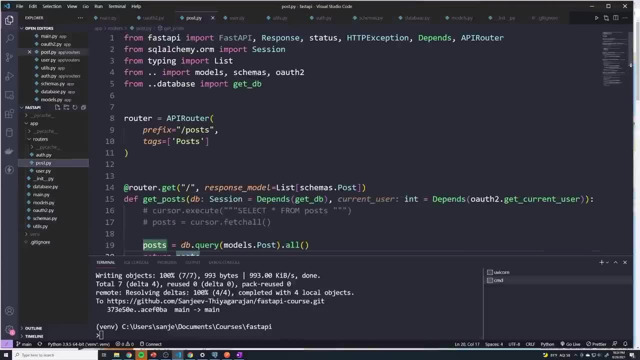 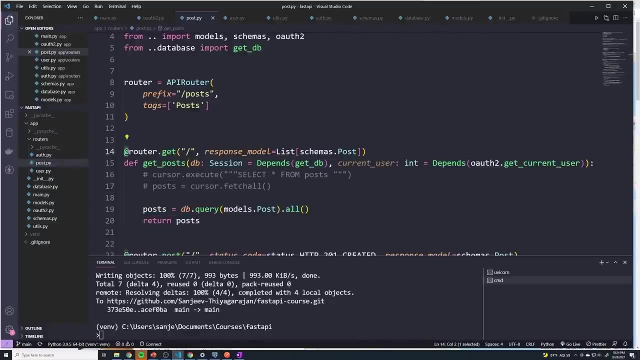 a couple of query parameters that they all use. So let's go to our app real quick, And what we're going to do is we're going to go to our post router And in this case we've got our path operation of retrieving all posts. And what I want to do is I want to let the user be able to kind of 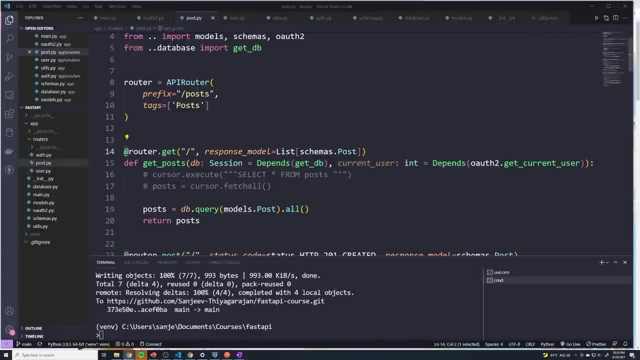 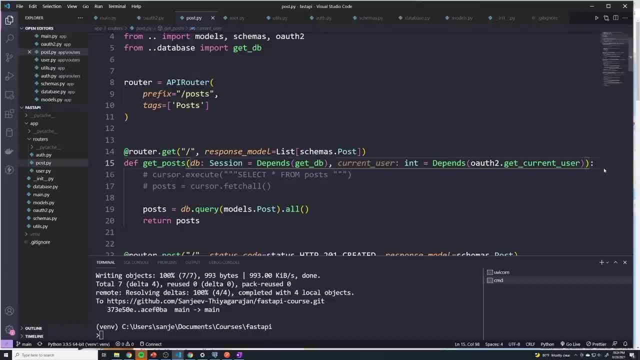 10 posts, or maybe I want 100 posts, or maybe I want 50 posts. we should allow the user to define that And so to to allow a query parameter, we could just go into our path operation function and just pass in another argument. So I'm going to do question mark, then we give it the name. 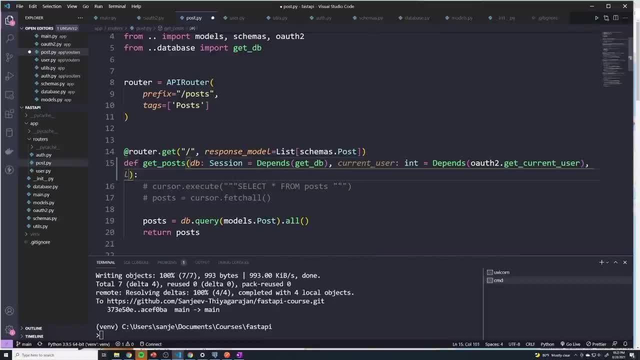 of the query parameter. So this is the key, essentially, And I'm going to call this limit. So this is going to limit the number of posts they get And this is going to be of type int And we're going to give it a. 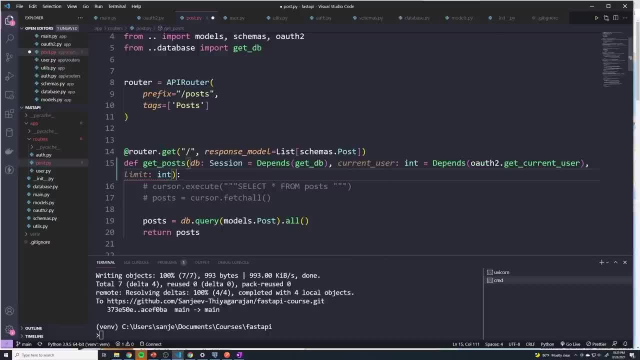 default value. So we'll say that you know, by default, if they don't provide a limit, we're going to say the limit by default is 10.. And now I'm all I'm going to do is I'm going to. 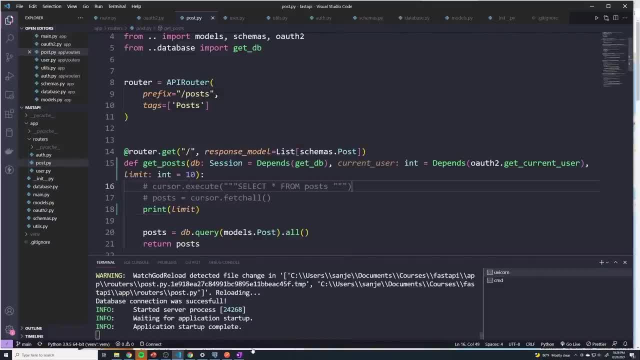 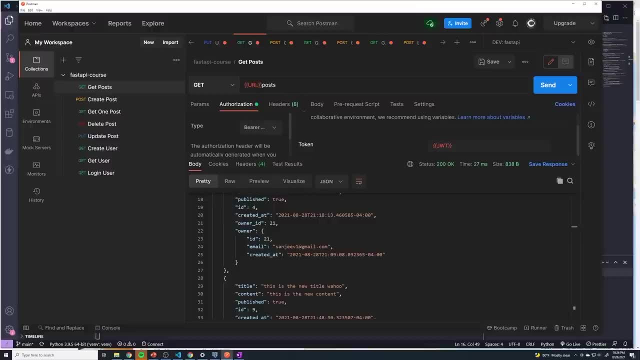 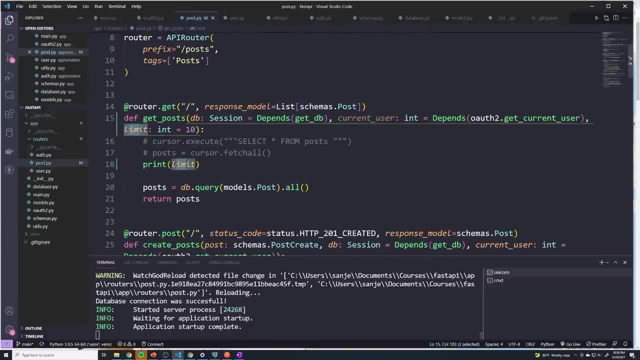 print out limit. All right, and I'll show you guys how to actually send that query parameter. So let's go to our get all posts And so to send a query parameter. it's very easy. you just type in a question mark, then you grab the name of the query parameter, which, once again, is limit. So 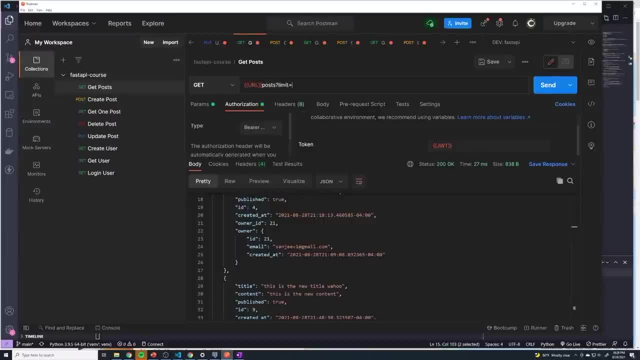 we'll grab limit. And then you say: if you set it equal to whatever value you want it to be. So if I want to get a limit of three, if I hit Send right, nothing should have changed in our code. But you can see. 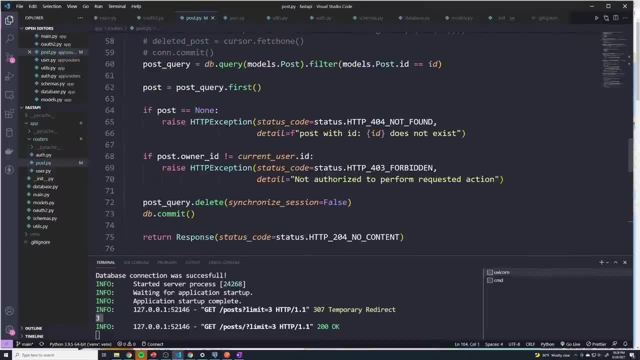 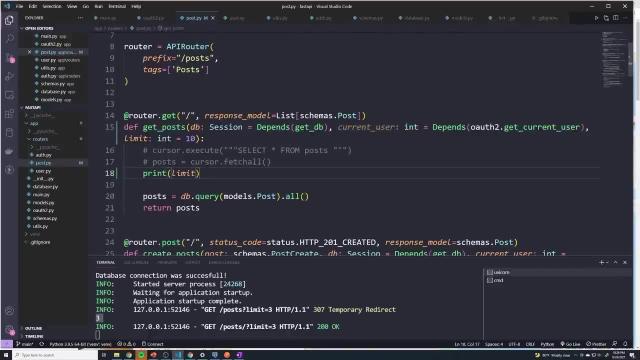 that we were able to print out the limit. So that's how we access query parameters in fast API. it's pretty simple: you just pass it in as another argument into your path operation function. But let's actually set up our query so that it now takes into account the limit. 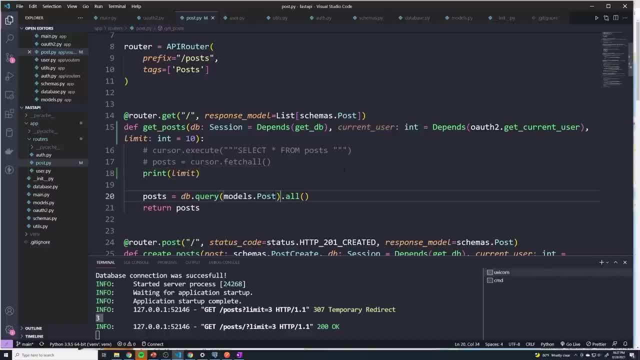 And with SQL alchemy, anytime you want to, you know, perform another operation, have a built in method. So I'm going to remove this dot all for now, And so if I want to limit the number of results, I just do dot, and then let's see what methods we have at our disposal. 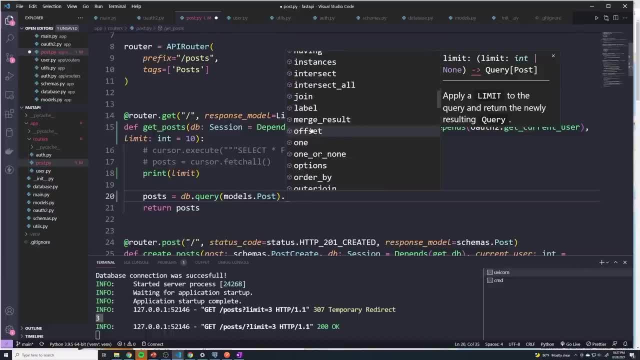 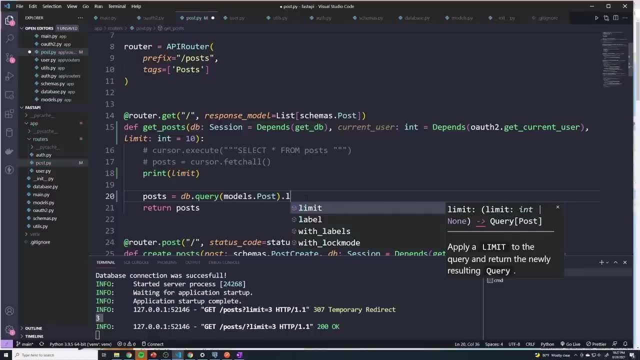 Since we're looking for something that limits something, let's maybe check to see if there is a limit method- And looks like I don't see one here, but there actually is- We can do limit, And then here I'm just going to pass in the limit variable. 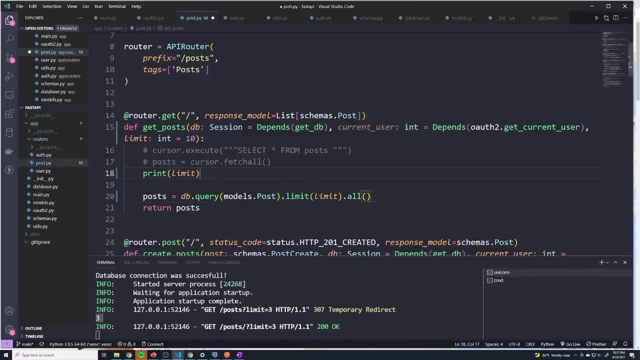 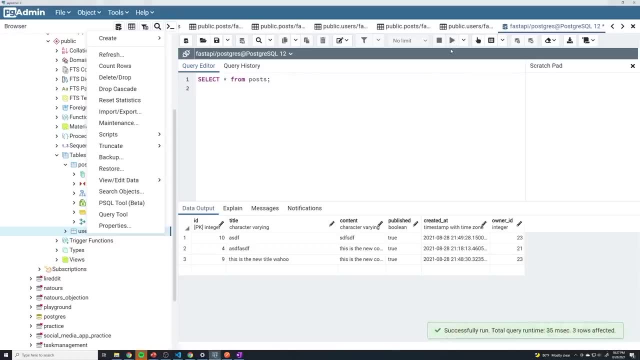 And then after that, we can just do the dot all, as we usually do. All right, and so now. well, first of all, in our database we don't actually have that many posts, So I'm just going to create a couple. Well, actually, I could just do this through. 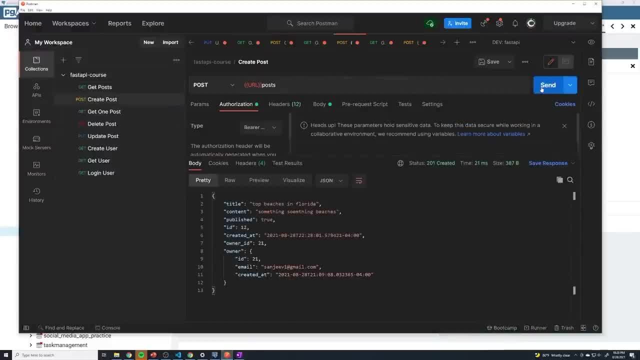 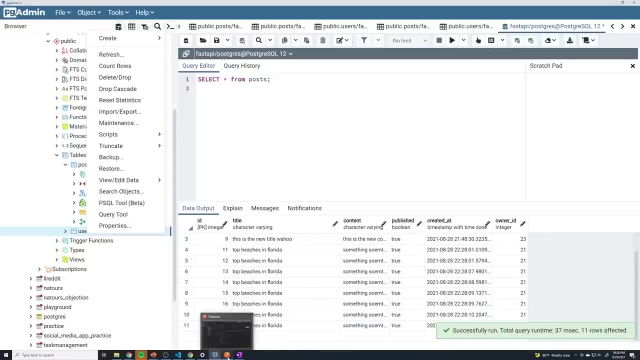 our API a lot quicker. So I'm just going to create a whole bunch of posts, And so that should give us five posts. Now let's create a few more, Alright, so we've got 11 posts now, And then we'll go back to our API. 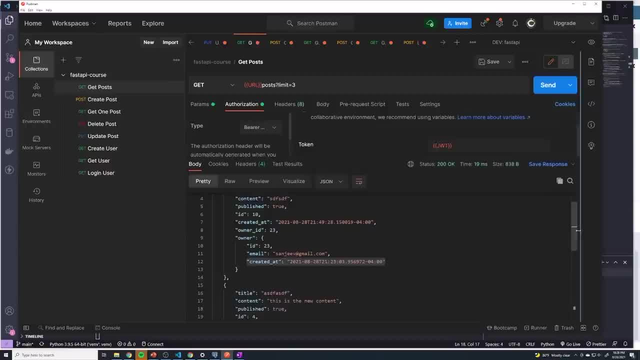 And we'll say: I want a limit of three, So let's send that And let's see. if we only get three posts, we get 123.. Perfect, And if I don't provide a limit, well, actually let's try a different. 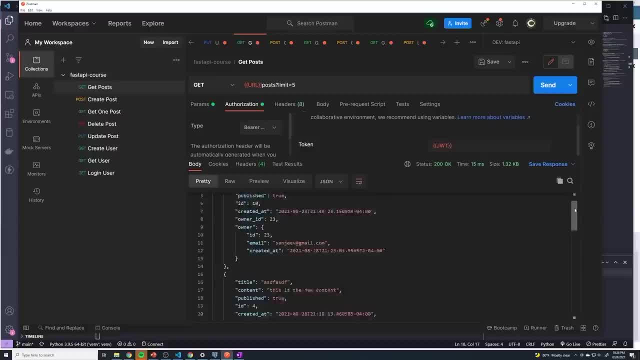 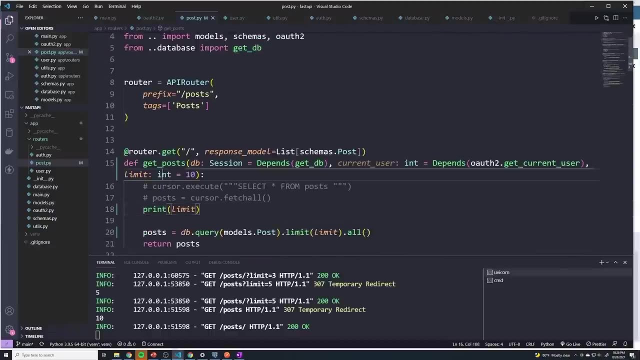 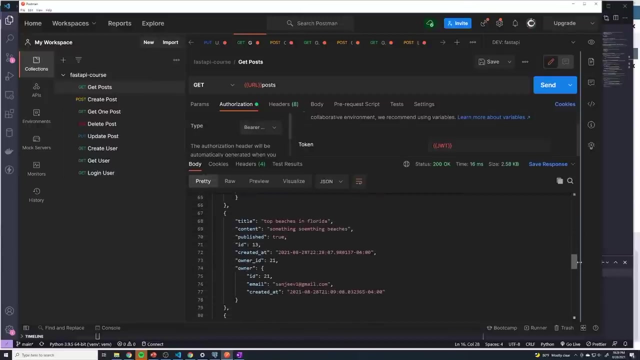 number. Let's try five now. All right, we get 12345.. Perfect, And if we don't provide a limit altogether, it should return 10, because our default was set to 10 posts, The limit is 10.. The limit of 10.. And so we get 12345678910.. And there are 11 results. So there's one result that 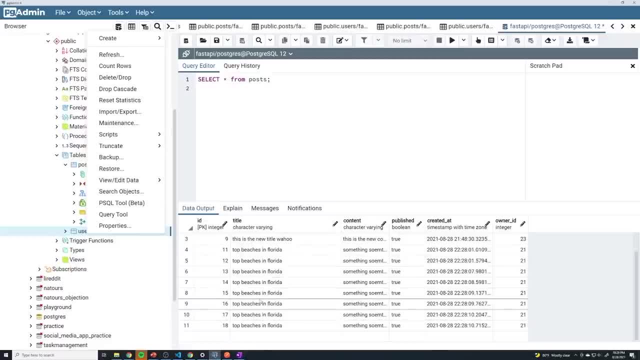 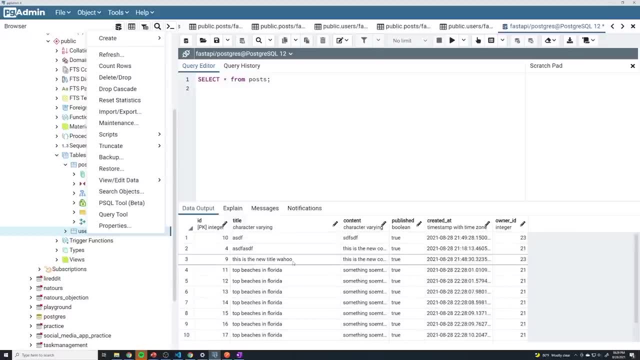 it didn't provide, So we've got the limit functionality down. What I want to do now is allow the user to skip results. So it grabbed, you know. depending on however Postgres has decided to return, you know, 10 posts. it grabbed the first 10 based off of some criteria. 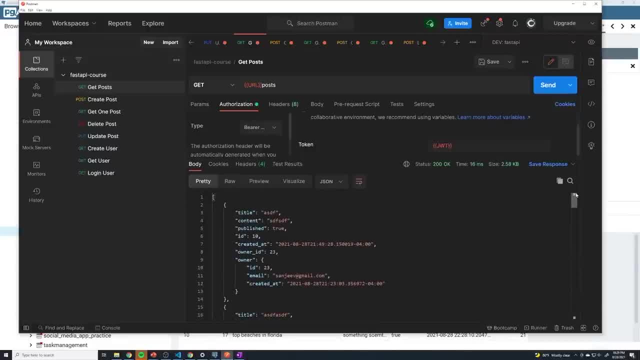 And if we actually take a look at how it looks like we got ID of 10, ID of four, so it's kind of just all over the place. So it's probably not sorting based off of any specific field. we may want to specify that, But what we're? 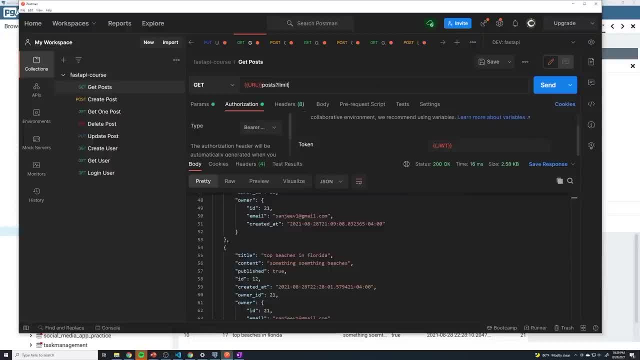 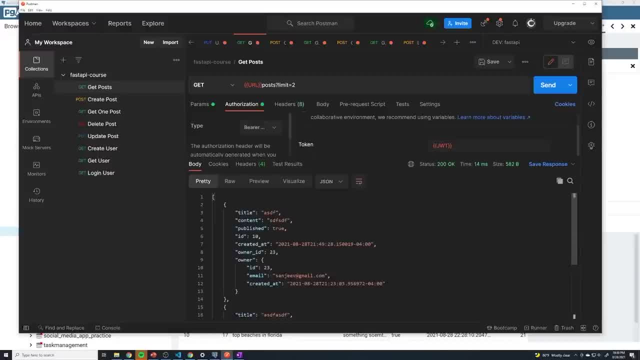 them. maybe we want to skip the first, the first two, maybe we want to skip these two. well, I want to be able to send another query parameter called skip, so that we can specify how many we want to skip. And if you want to send more than one query parameter, we just do the end keyword. 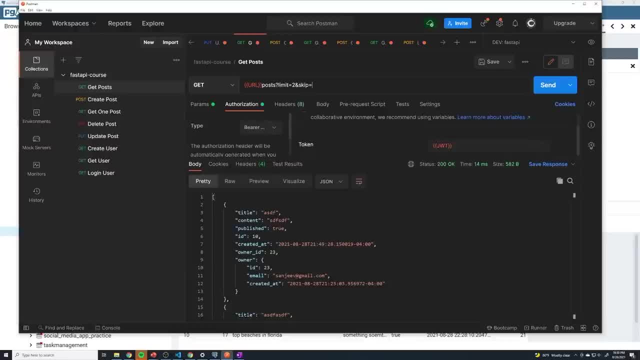 and then we provide the next key value: pairs. it would be like skip equals two, And so, just taking a look at the IDs here, we've got one with an ID of 10. And one with an ID of four we want to skip. 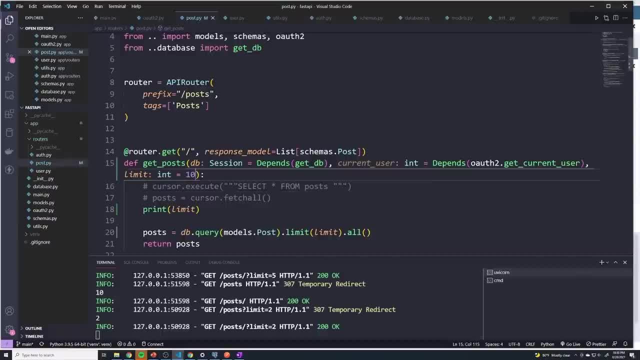 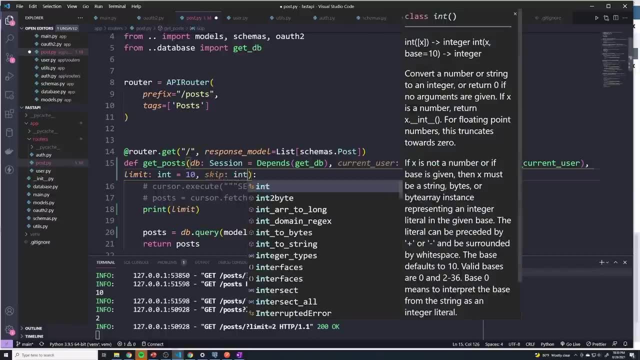 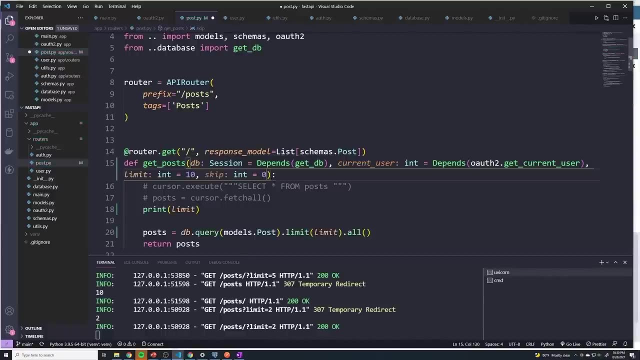 both of those. So, going back to our code, we're going to provide a another path operation function. sorry, another argument into the function, and we'll call this: skip is going to be of integer and the default is going to be, we'll say zero, we don't want to skip anything by default And to 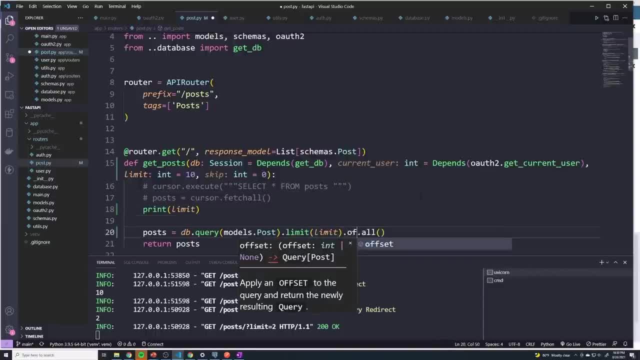 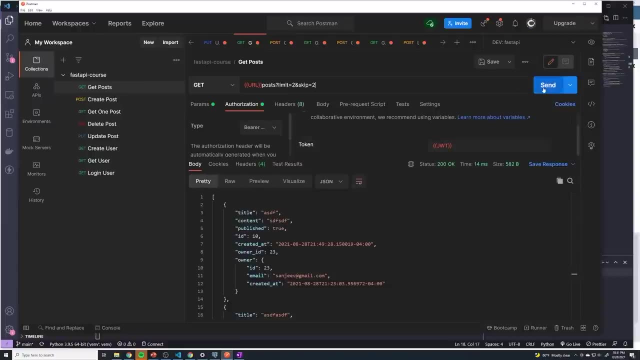 add this to our query. we use the keyword offset, we do offset, And then here I'm going to say: offset equals skip, All right, and so we should be able to skip over both of these, And so if I provide a skip of two, you can see it first starts out at nine and then 11.. 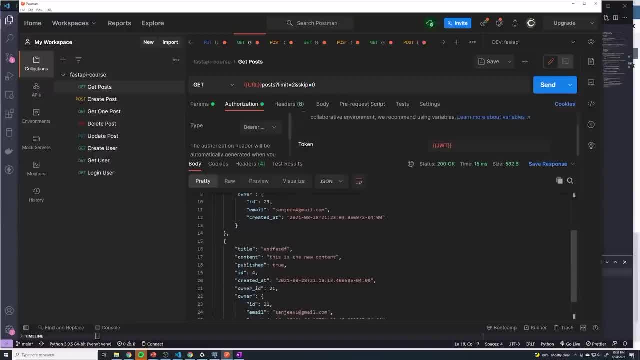 If we do skip zero, it shouldn't skip any right 10.. And then an idea for if we skip one, it should just skip the 10 and then start off on four, And we can see that the first one is four, So it allows us to skip over, post that, And so that's ultimately how we're going to implement. 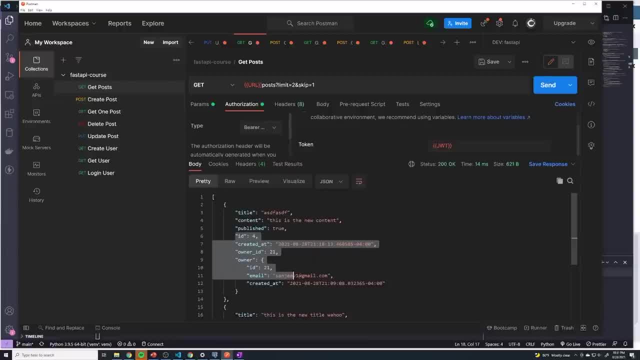 pagination on the front end is because the front end should be able to skip based off of what page they're on. So if each page returns 20 results and you want to go to page two, then you want to skip 20 results. If you want to go to page three, you would skip 40 results. 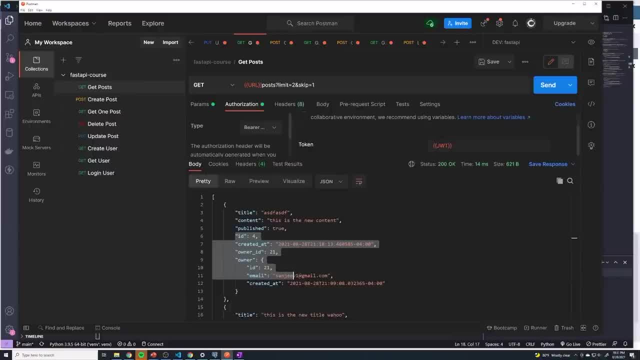 Now, the last query parameter I want to set up is a search functionality. I want the user to be able to search based off of, you know, some keywords in the title or maybe even the content, depending on how we want to implement searching. For for now we're just going to say we'll be able to search. 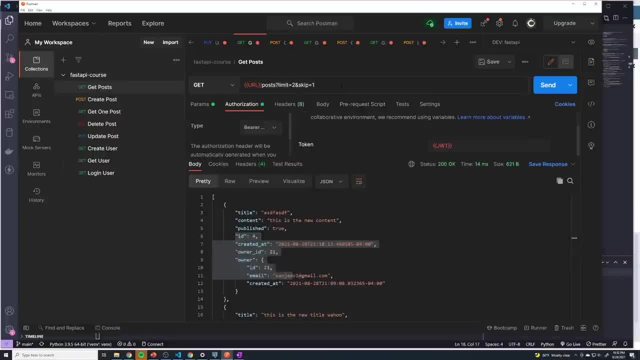 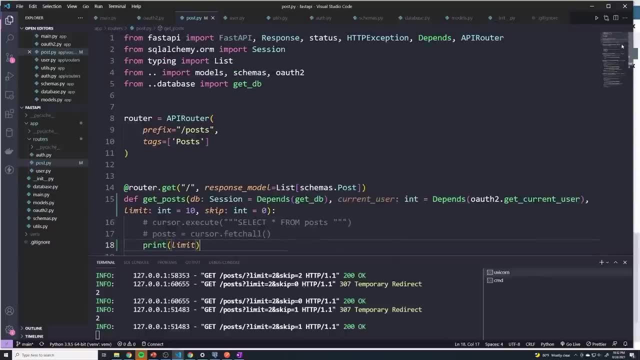 based off of the title, And the way that the search will work is we'll have another and and we'll say: search equals, and then you know some random text, And so, once again, we're going to provide another argument called search, And this is going to be of type string. However, this is. you know, we can't. 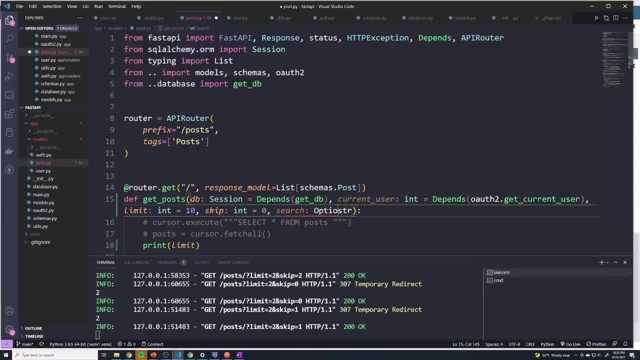 exactly give a default search. So I'm going to say this is a optional, It's gonna be an optional string, but we don't have to provide this And the default is just an empty quotes And it looks like I have to import optional from fast API or from typing. 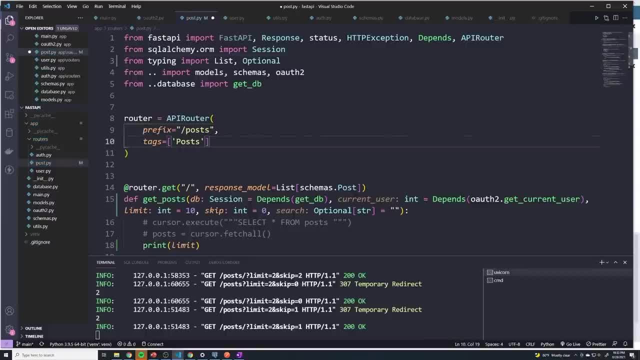 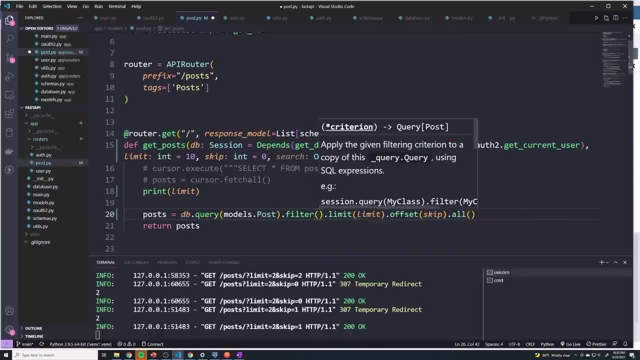 And so here I'll just say import optional, And this is going to give us an optional query parameter. And so what we're going to do here is I'll say filter And to filter this and just kind of like how we filtered based off of a specific user ID or a specific post ID, I can say: 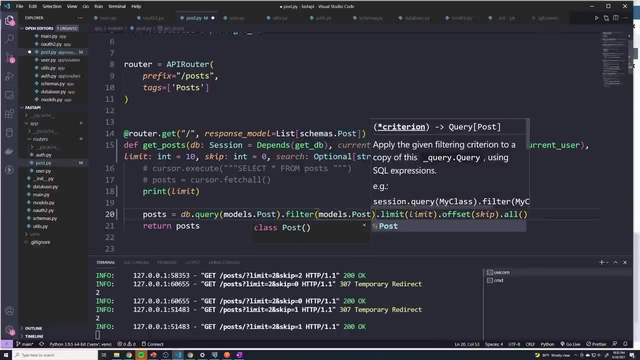 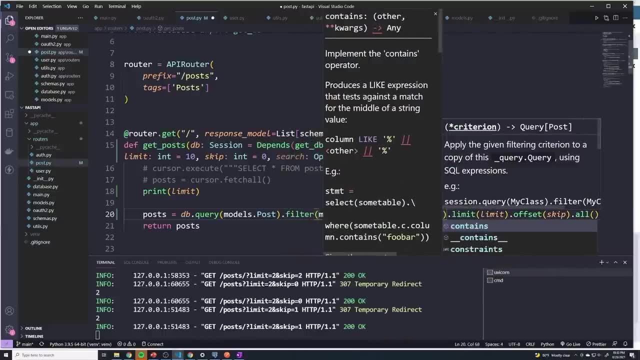 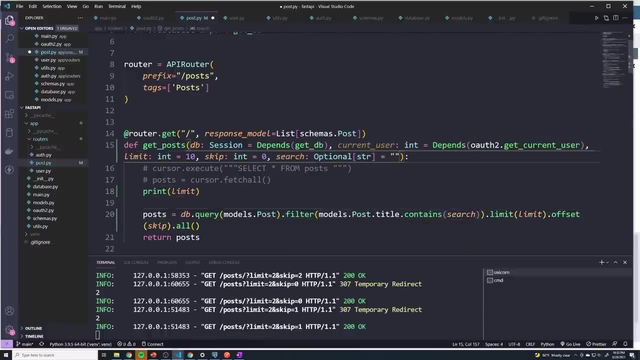 models: dot, post, dot title, And then we can use a method called contains, So we can say contains and then the search keyword. So this will allow us to provide some kind of string and it'll just search for the entire title of a post And I'll see if the search 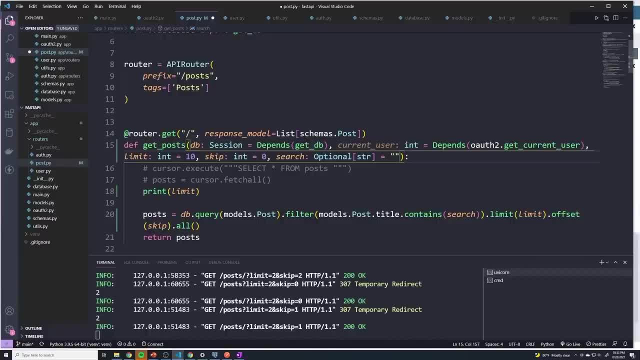 keywords are anywhere in the post title. it doesn't have to match completely, it just has to be somewhere in the post. So this will give us a little bit of flexibility. So we don't have to match the exact name of the post. we could just provide some keywords like: 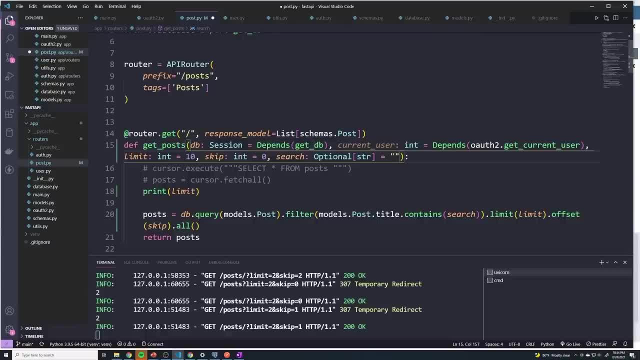 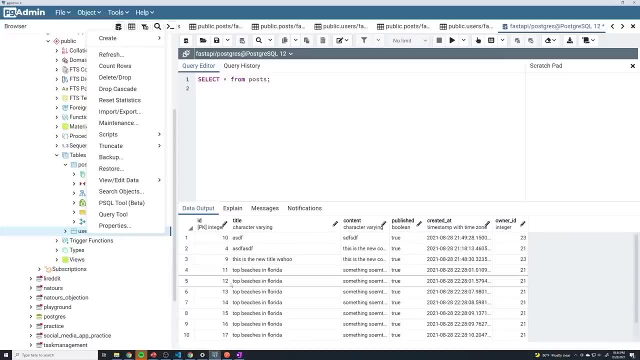 like hot dogs or beaches or whatever, And it should be able to just see if it's contained in there. So let's take a look at our database. You can see that we've got a lot of ones that say top beaches in Florida. So I'm just going to do a search And if I just search for beaches, it should. 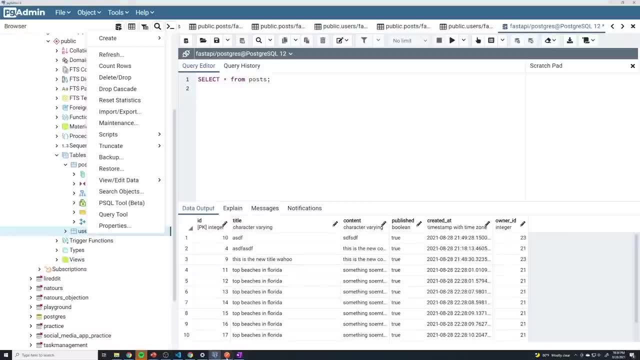 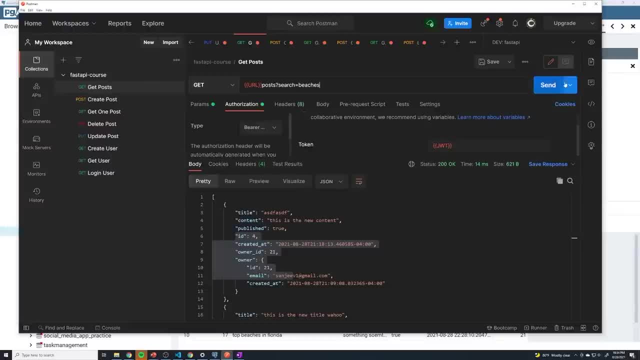 return all of these because they all contain the word beaches And I'm just going to do a search And I'll get rid of the limits and the skip, for now We don't really need that And all of the results should be: actually. I don't think I saved it, Let me, let me save that And now, if I do this, you can see that. 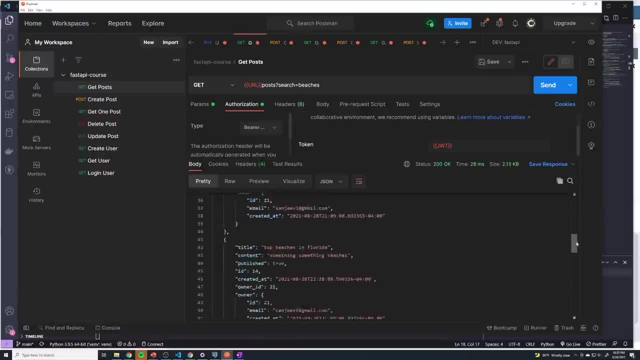 every result is going to have the word beaches in in the title, And when it comes to query parameters, you can string as many as you want. So if you wanted the limit as well- and we'll set the limit to two, And we can also provide a skip- 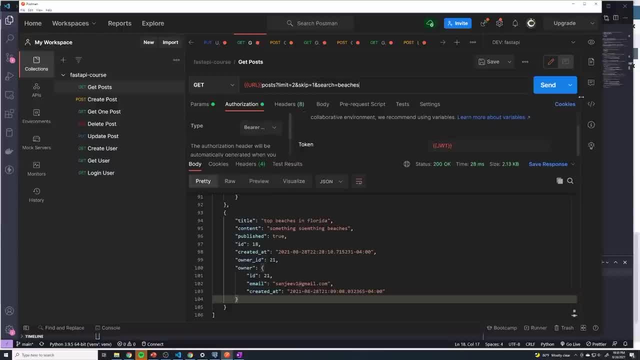 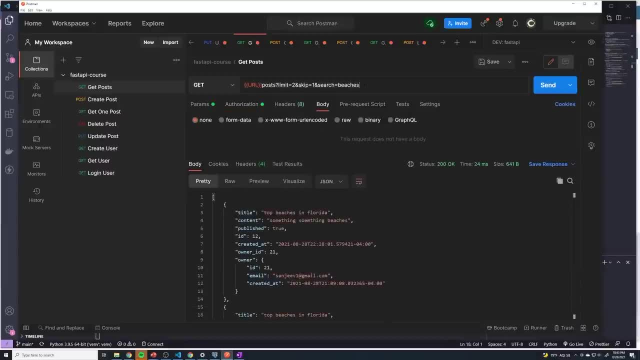 Equals one. you can add as many of the query parameters that you want, So now you can see that we set the limit to two and we skip the first one. Now the last thing I want to show you guys is how to use spaces in your search query, Because right now we just have the 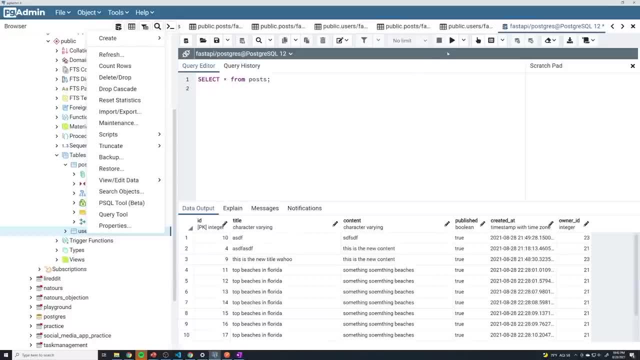 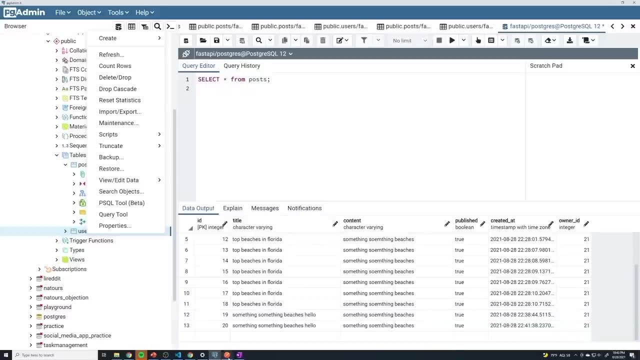 word beaches. But let's say I wanted you know. just going into our Postgres database, let's see what I've got. Maybe I want to search for beaches, Hello, or something: beaches, right, How do I, how would I search for that in a URL? I can't put a space in the URL. I can't say you know something. 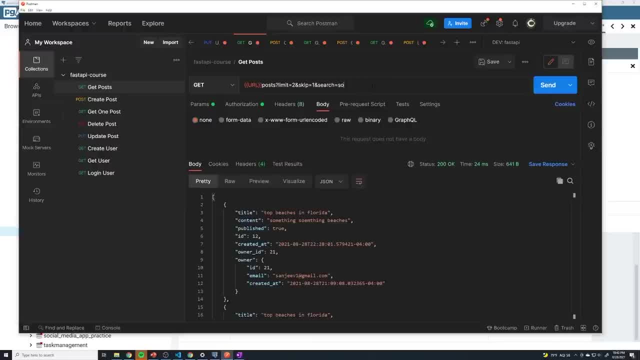 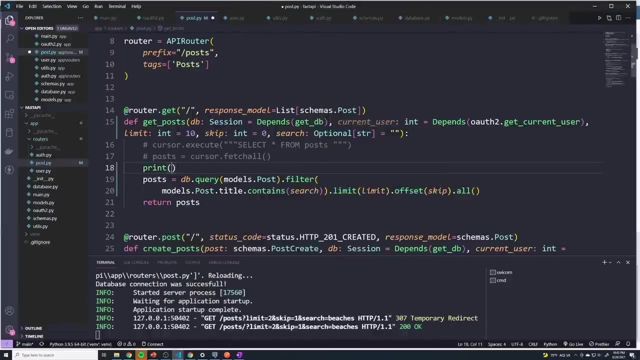 beaches. So how do I do a space? Well, I can do percent and 20,, which is reference, which means space in your URL, And then you can do beaches. So then, just to verify that that's actually returning what we want, I'm going to do a print. I'm going to print out the search keyword. 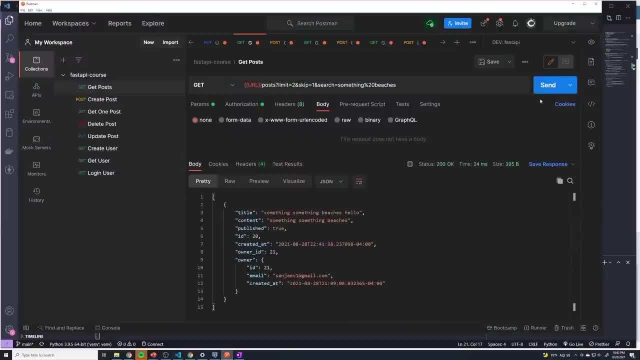 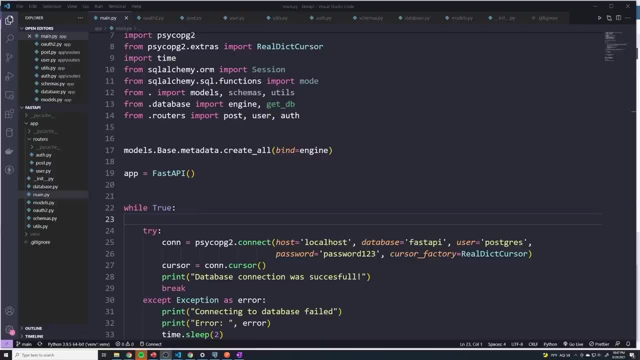 And we're going to test this out. So if I hit send, you can see that it returned the one result that has the word something and then beaches, but it doesn't return anything else. What I would like to do now is do a little bit of cleanup on our mainpy file. you'll see that there's a lot. 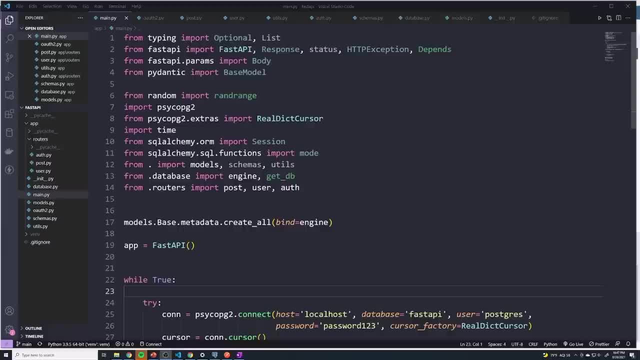 of unnecessary imports that we don't need, especially since we moved all of our routes into their respective folders, So you'll see that a lot of these are grayed out, And so anything that's grayed out we can move above. before we actually do that, What I actually want to do- 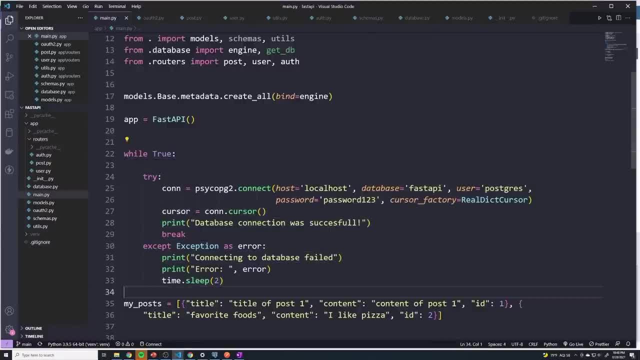 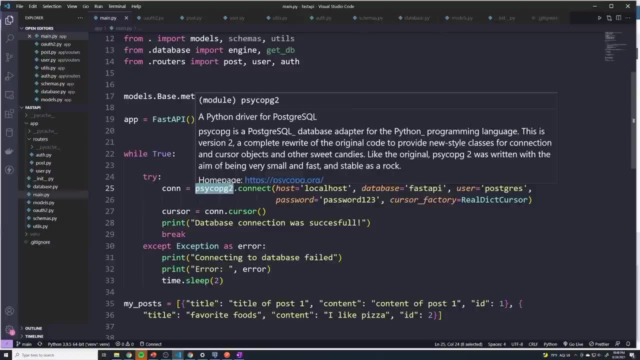 first is: I want to take this code for connecting to our database using the. you know the regular code that we have in our database And I'm going to take this code and I'm going to move that to our databasepy file And keep in mind we can just delete this because we're no. 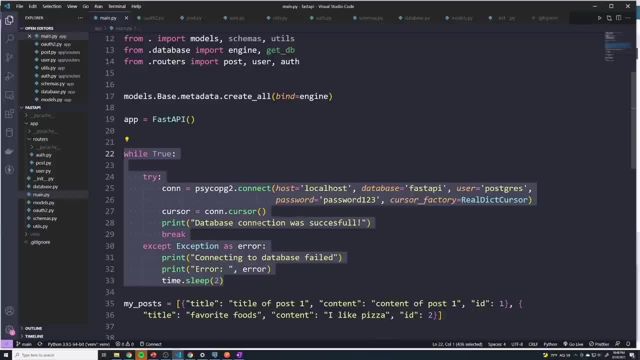 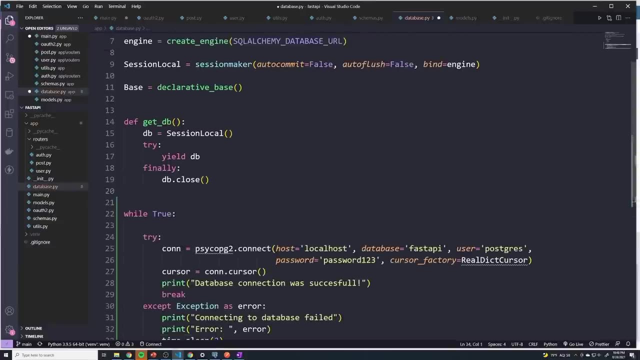 longer using this And we're using SQL alchemy to actually connect to our database. So you can actually delete this. But just for documentation purposes I'm actually going to just cut this out And I'm going to move this into our databasepy file, Just that you guys have this for reference. 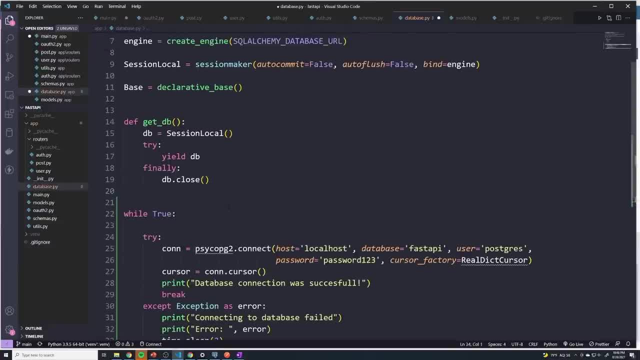 in case you ever want to, you know, run raw SQL directly using this Postgres library instead of using SQL alchemy. I want to make sure this course covers as many different you know possible situations for you guys, But moving this here, obviously we're going. 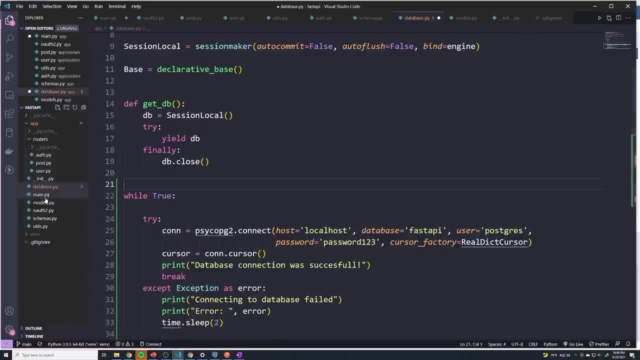 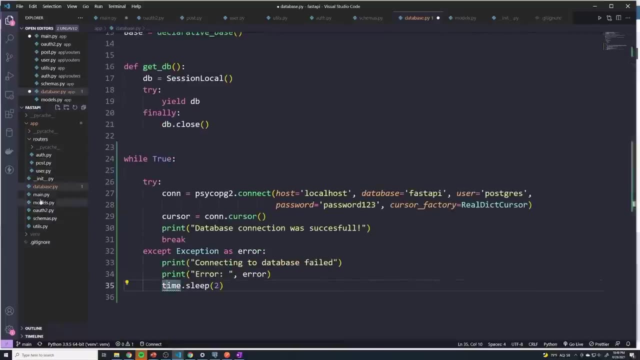 to get some errors, because we have to import all of these And I'm just going to go to our main and I'm going to import them from here. So here I'll just copy these two And we'll actually just cut it out, And then it looks like we also need time. where is that coming from? 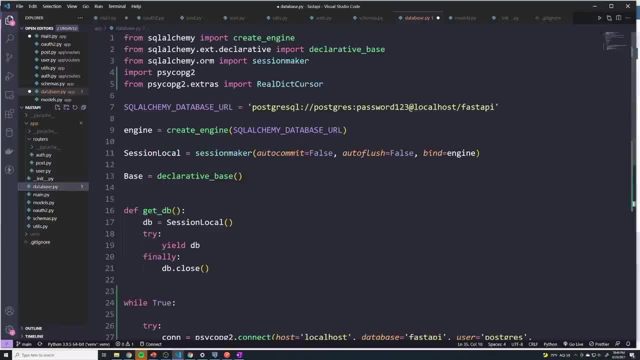 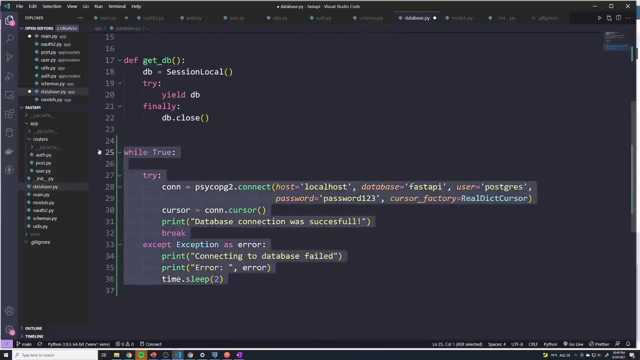 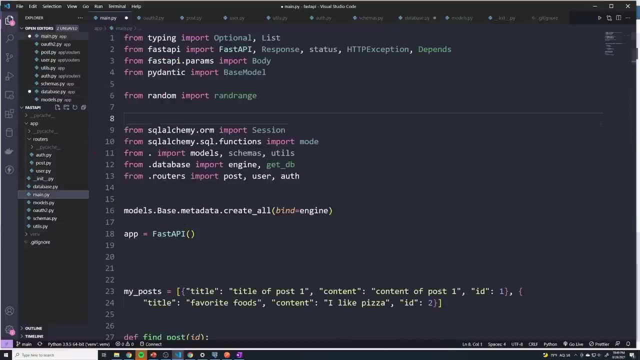 It's just coming from the time. Okay, All right, that should remove any errors And we can just comment this out, actually, because we're not going to use that anymore. And then, going back to our main, you can see that both of these are. 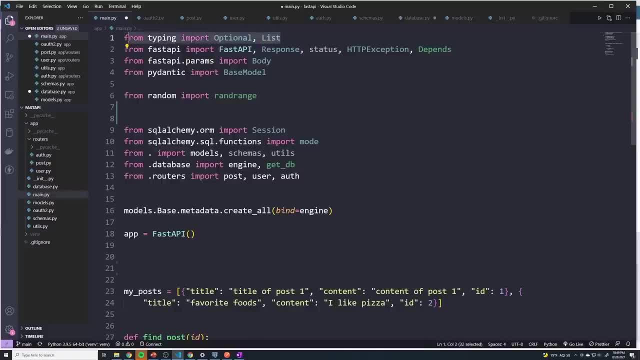 grayed out. So we're not even importing anything from typing anymore, or we're not using anything from typing, So I'm going to remove that. You can see that we're no longer using status, So I'll actually. we're no longer using all of these, So I can remove all of those And I'm not using the body. 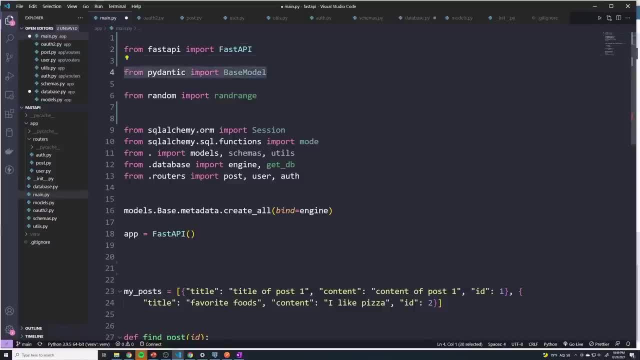 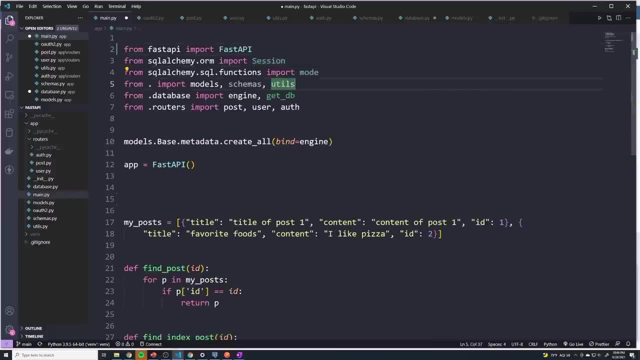 here anymore. I'm not using anything from pydantic And I'm not using anything from random. We'll just get that a little bit closer. We're not using session anymore either, So I'll remove that, This, whatever that is going to remove that, And then we'll remove schemas and utils. 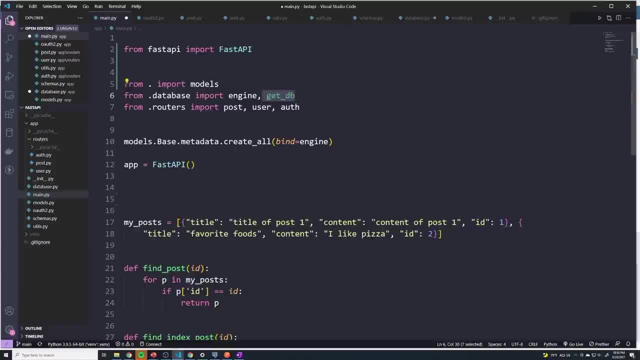 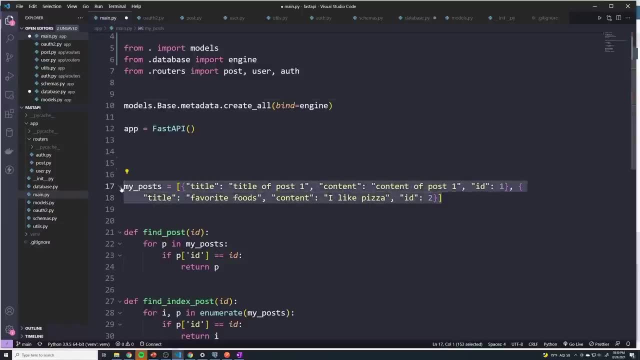 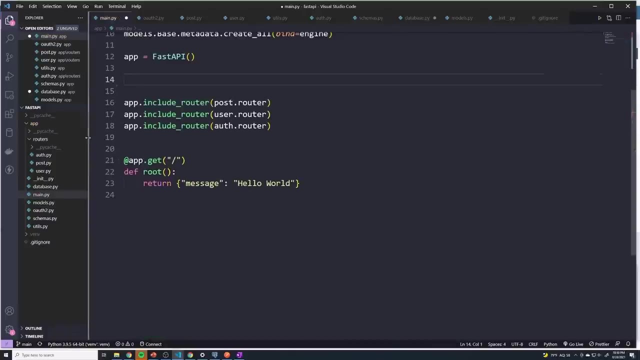 We can remove get DB as well, And then obviously the the posts array or list, that's no longer needed. These two functions, they're no longer needed. They were before we started working with databases And then I mean we don't actually need this route anymore. But I'll just leave that. 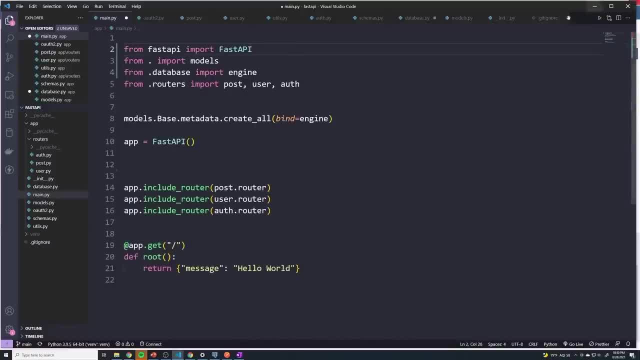 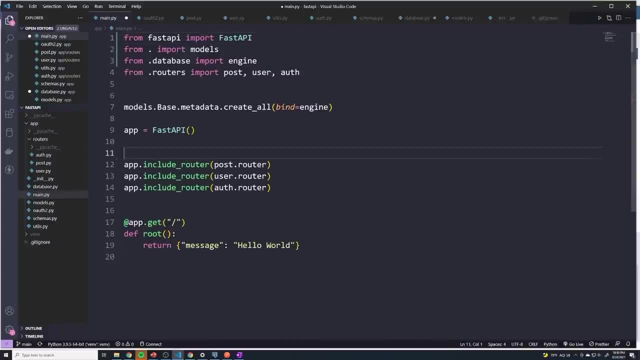 in there, But you can see that our code is a lot cleaner now after removing all of those unnecessary imports. I'm just going to structure this a little bit better, So all the codes a little bit closer together, And I think that's all the cleanup that we need to do for now. I just 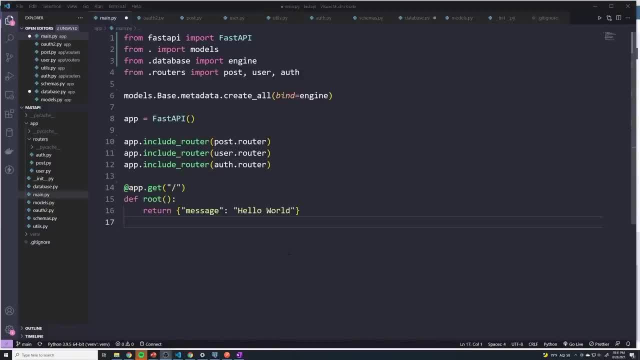 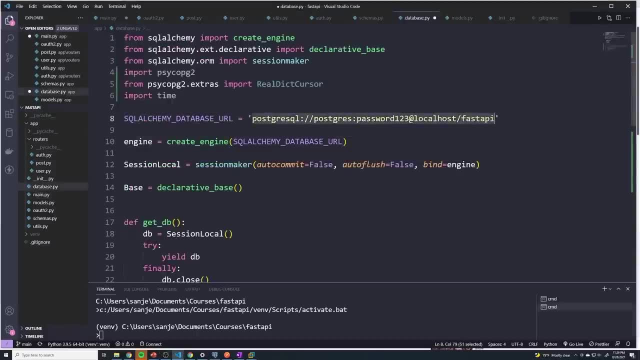 wanted to make sure there wasn't too much garbage building up in our application. When we first started working on databases, I mentioned that we should never hard code our database information or the database URL into our code, Because this creates two issues. First, 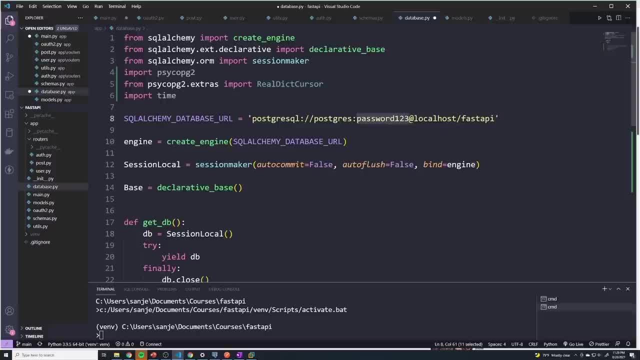 of all, we're exposing our username and password right there in code So anyone can see it. if we check it into GitHub, Anyone who has access to it can see our password now, And at that point we've compromised our application. But on top of that, the other big issue is: 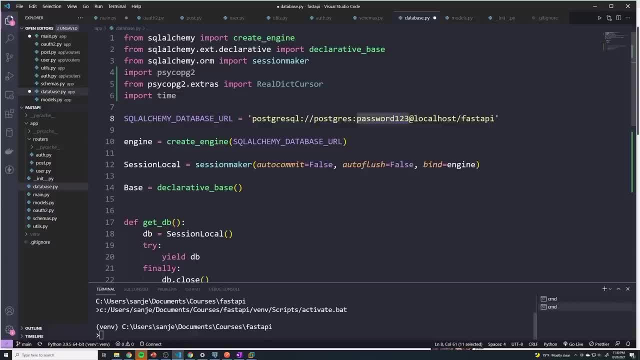 that right now we've set this URL to go to our development Postgres instance, which is running on our local machine. When we actually deploy this to production, our Postgres server is not going to be running on this machine. It's may not even be running on the machine. 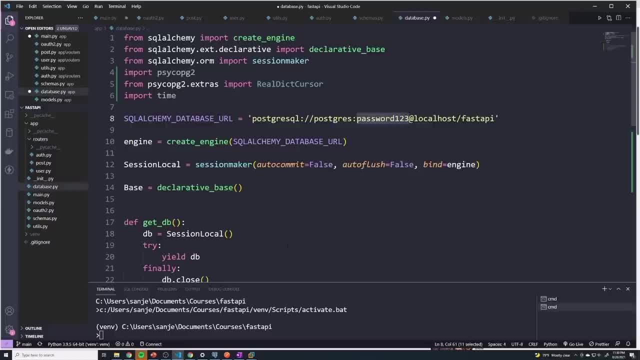 that our application is actually deployed on it can be on a completely different system, So we would need a way for the code to automatically update in a production environment to point to the actual production system Postgres database, instead of using the one that's hard coded in here, And so we need 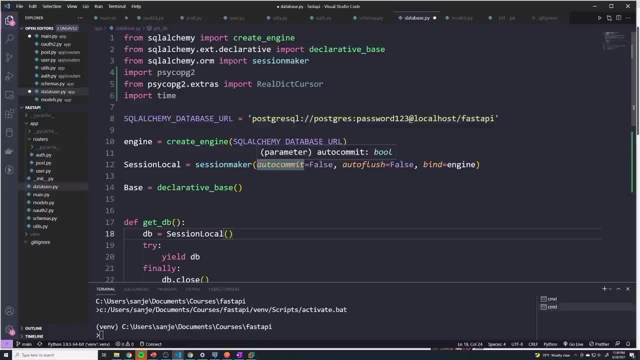 a way to do that, And keep in mind this: this isn't exclusive to just working with the databases. any kind of confidential information, any password secrets, anything that needs to get updated based off of the environment that it's in, needs a way that will will run into. 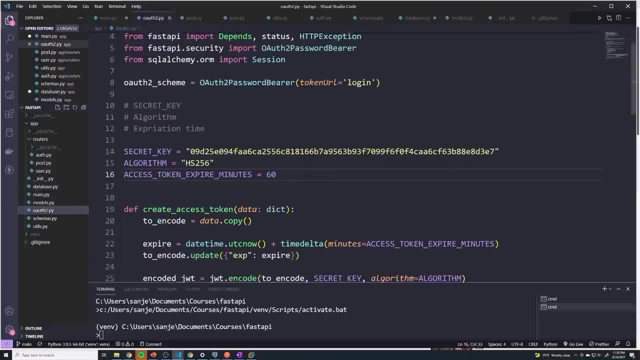 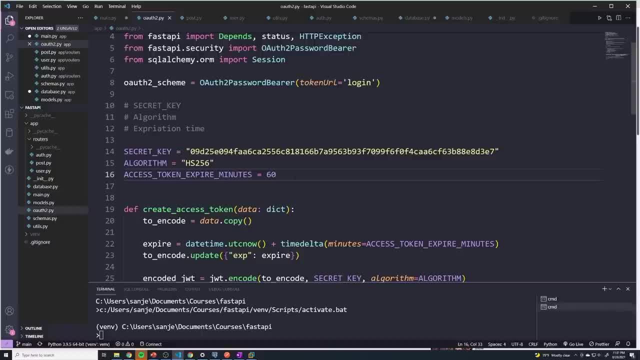 going to need a way to do that, And so we're going to need a way to do that, And so we're. you know, whatever, like we might have an environment variable called Postgres underscore URL and that's going to contain the URL of our Postgres database, And so we don't need to hard. 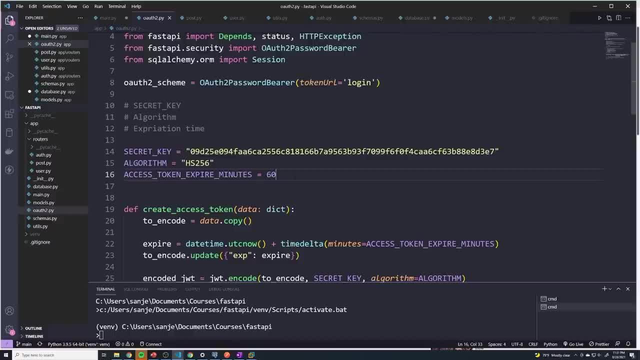 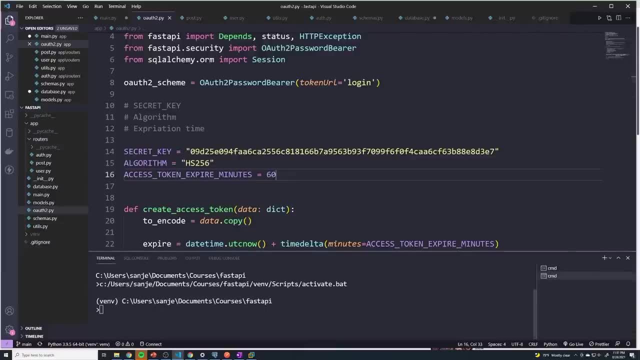 code the actual value. we hard code just the name of the variable, And then Python will automatically pull in that variable. So let me show you guys how to do that, And I'm going to show you guys how to do this on Windows first, And then we'll take a look at this on a Mac or Linux machine. 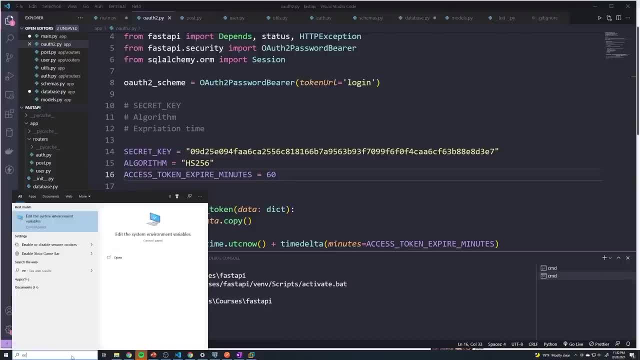 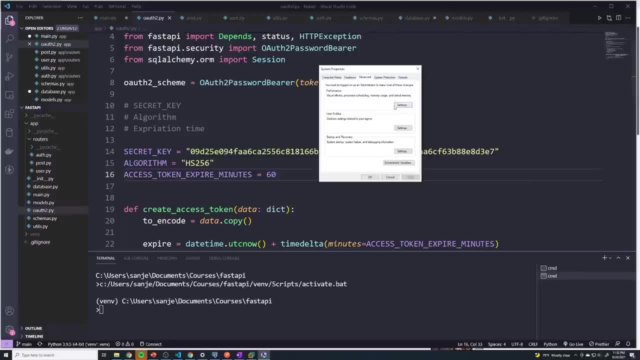 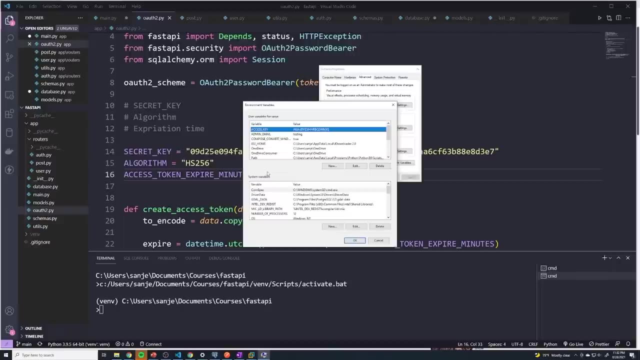 Mac and Linux are the same steps. So I'm going to search for environment And you'll see this: edit the system environment variables. And what we want to do is we want to go to environment variables under the advanced tab And here you'll see two sections. you've got system variables. 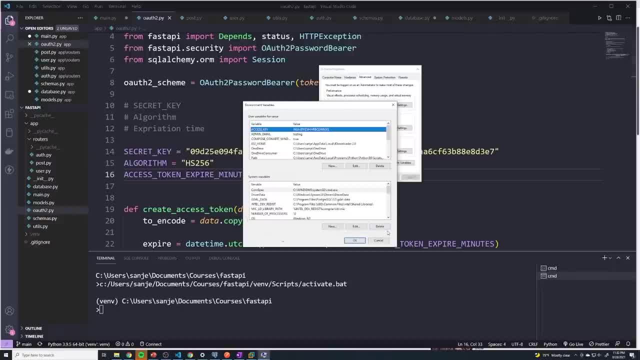 this is going to be environment variables that are system wide, which means any user can access them, And then we have a user specific variable. So these are variables that only I can access, And you can just, kind of, you know, go through these and just take a look at them. 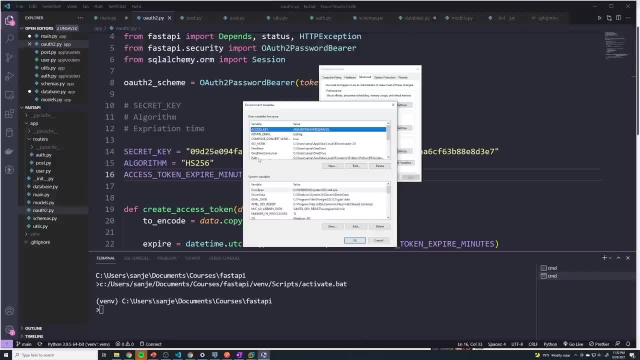 But you can see that we have an environment variable called path. don't worry about what it's used for. This is something that gets set up when you install your machine. But we're going to take a look and try to access this So you can see that this is the key: the variable name, path, and then 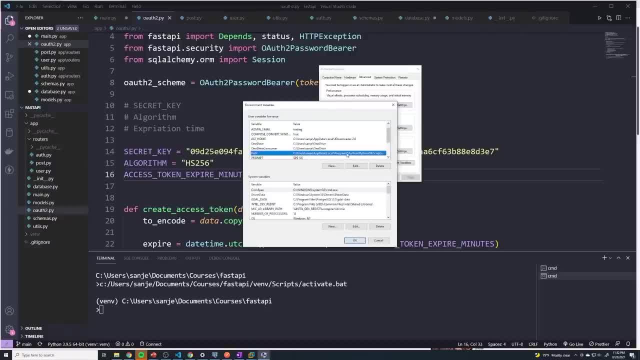 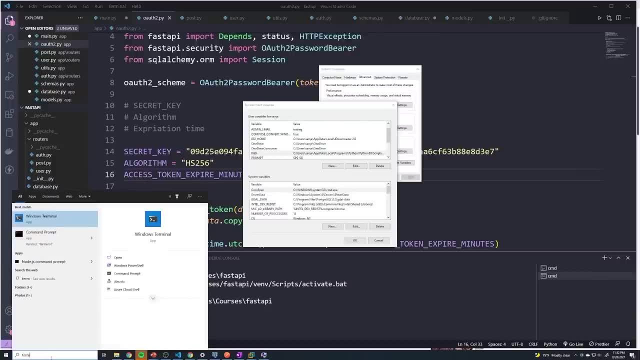 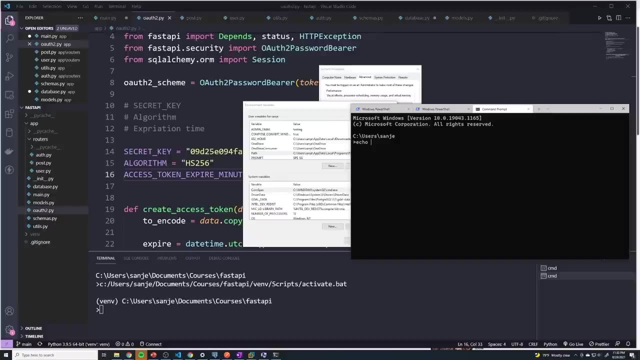 the value is some sort of path in our operating system or in our file system. So how do we actually access that? Well, let's open up a terminal, And here I'm just going to type in echo, And then we want to access an environment variable just to percent, and then the name of the. 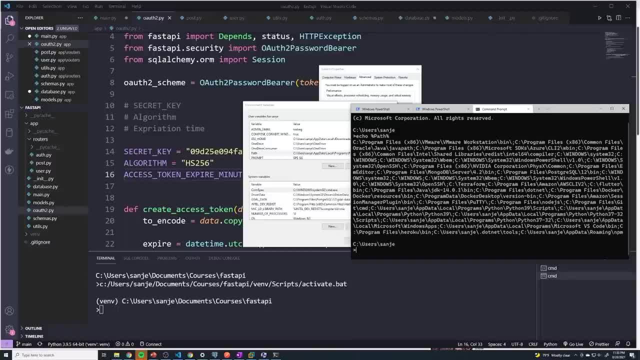 variable. So I'll say path with a capital P, And if I run this you can see that it prints out that specific path, And so that's how you access an environment variable on the command line With Python code. it's gonna be a little bit. 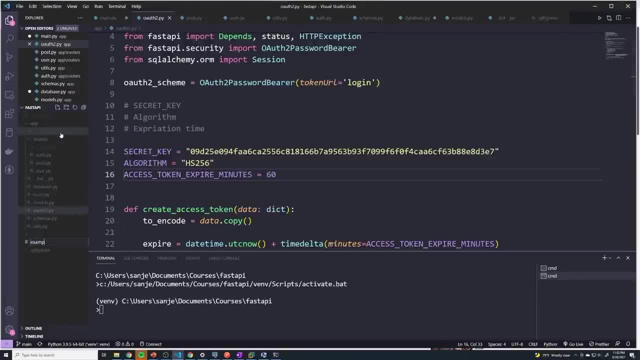 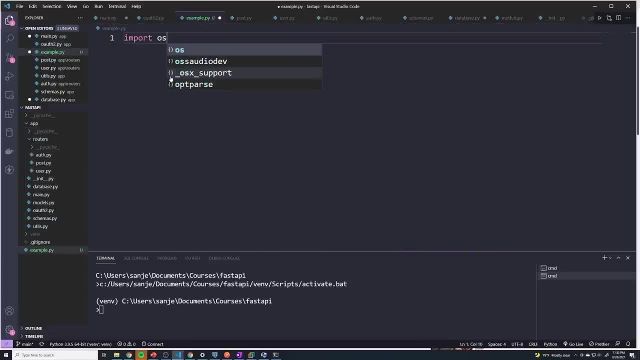 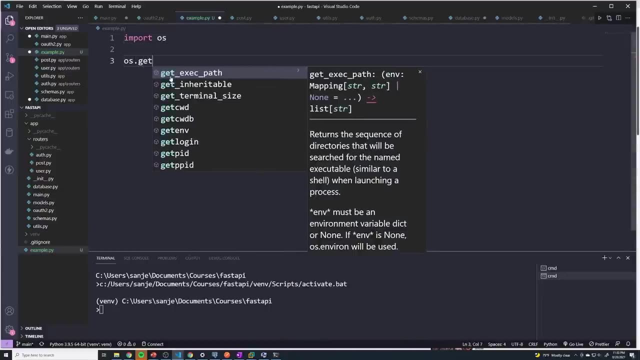 different, but it's still pretty simple. I'm gonna open up a new file Just for demonstration purposes. you don't have to actually follow along on this, And to actually access a environment variable we have to import the OS module And then to access that variable you say OS dot, get n v. 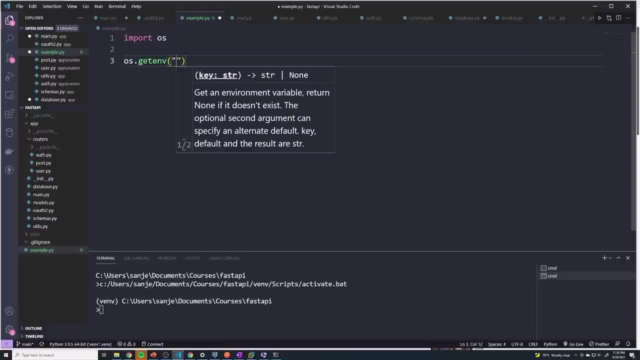 And then, within this method, you just pass in the name or the key of the variable. So in this case it's path And I'm just going to store this in a variable And we can call this anything. I'll just call this path, why not? And then I'll print out path so we can see how they see if it actually 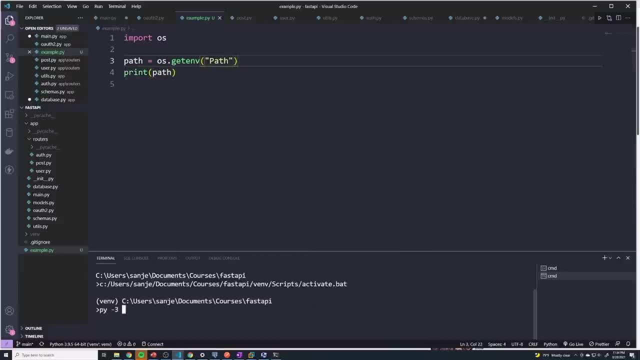 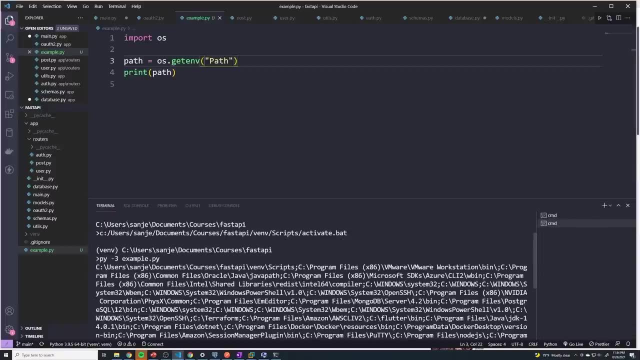 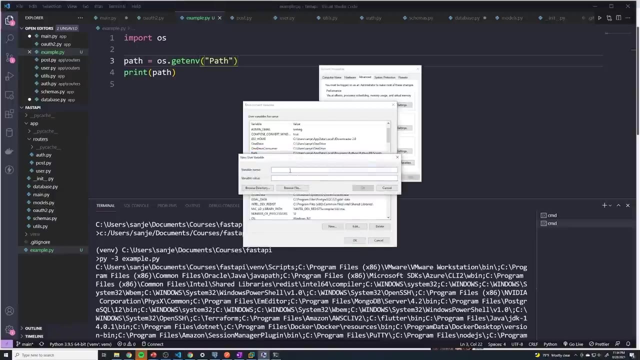 works. And now, if I do pi dash three and then run example dot p y, you can see that it printed out that same exact path. Now to set a new environment variable, we would go to new And maybe I create a URL, a variable name called Postgres, Or we can just call this: How? 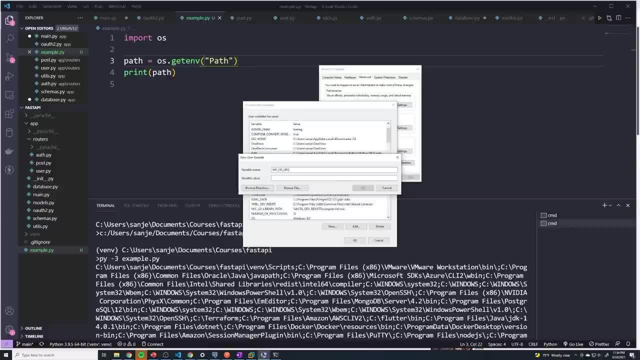 about my underscore DB underscore URL. So this is going to have the URL to access our database. I'm gonna say this is that localhost, colon 543.. Two, I think that's what our database is running on And I'll hit OK. And so here we can see that this is our new environment variable that we 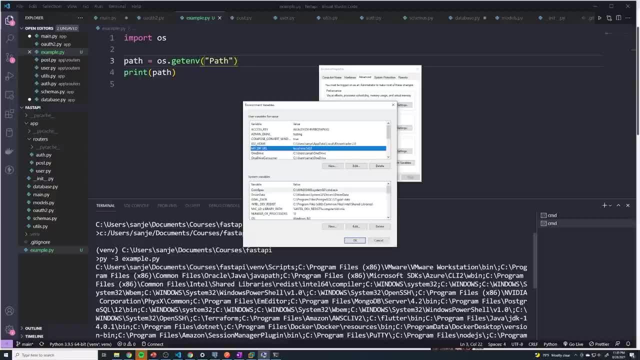 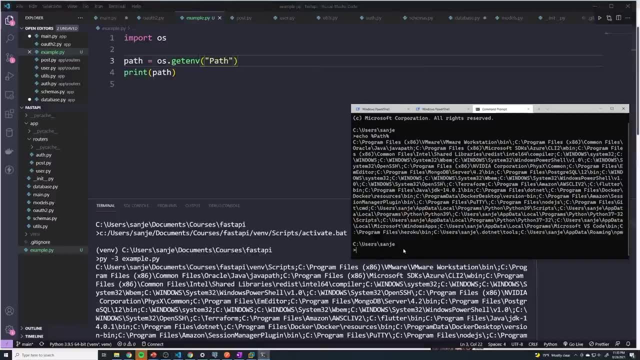 created my DB underscore URL and it's set to localhost five, four, three, two. I'll hit OK And I'll hit OK here And then what we're going to do is we're going to try to access that variable. So I'll do echo my underscore DB underscore URL percent, And actually it should. 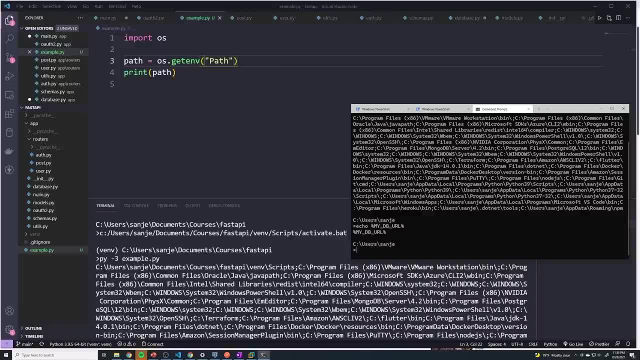 be percent, percent, And you can see that it does not print out what we said, it just prints out exactly what we wrote. So what gives what happened here? Well, anytime you set a new environment variable, what you got to do is you got to close out your terminal and open up a brand new one. So 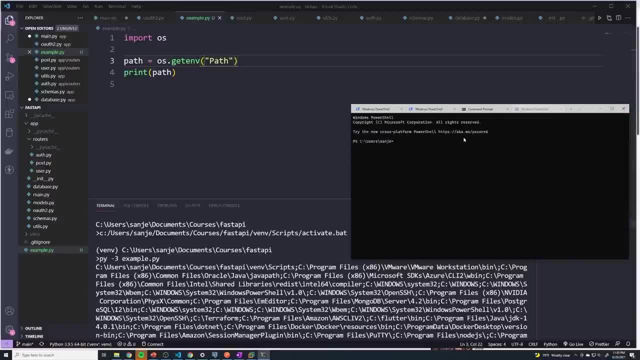 I can. you know, I can close this out or I can just open up a new one. And this new terminal. well, actually, I don't want to PowerShell, I want a command prompt. So this new terminal will be able. 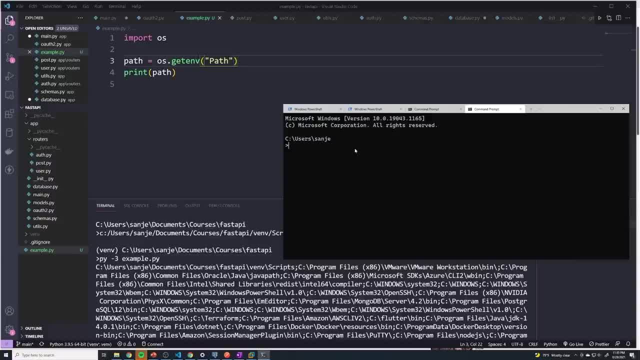 to access newly created environment variables because they get set as soon as the terminal opens. So once the terminals open I can't change them, So I have to open up a new one so that it can reread and import all of those environment variables. So now, if I do echo percent, my 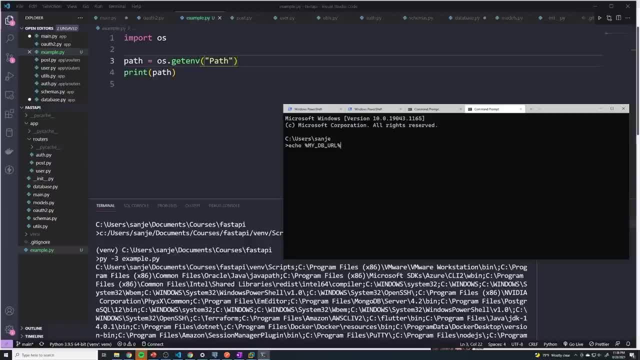 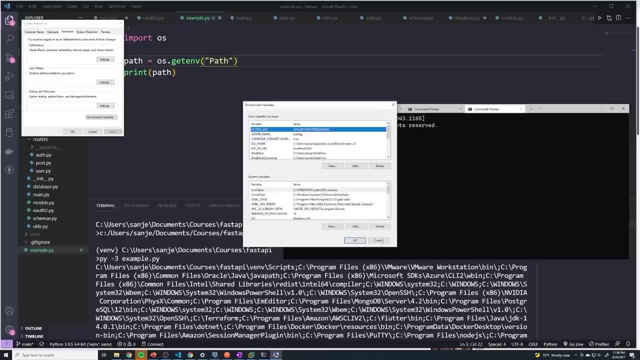 underscore DB, underscore URL percent. it looks like I may have mistyped this, So hold on, let me see what what is called, And that looks like it's correct. So what's what's happening? Well, I'm going to close out all of them, That's. 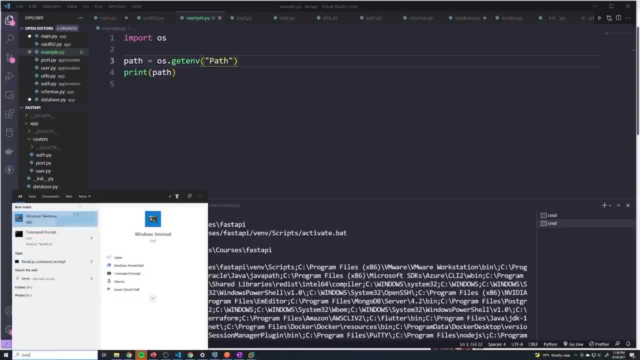 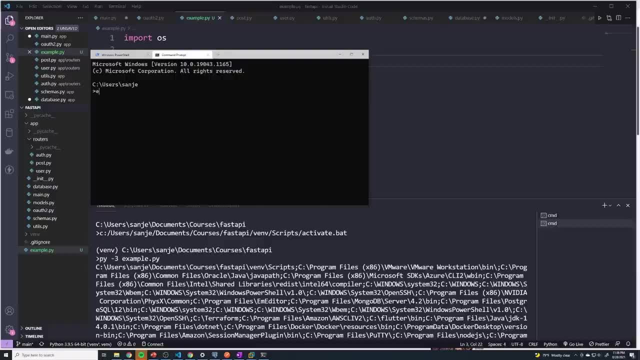 probably what's the issue. So let me open up a new terminal Now, open up a new cramp command prompt And now I'm going to try echo percent my underscore DB, underscore URL, And now we can see that we can read it. So we have to close out our. 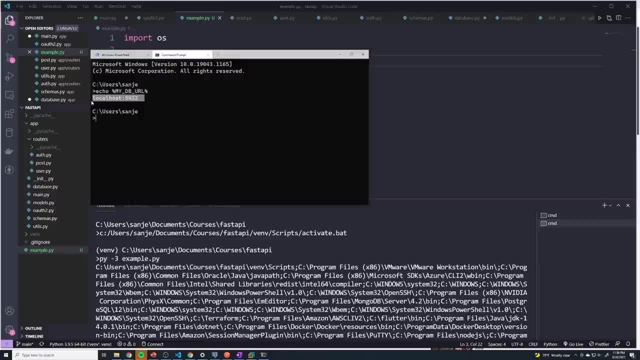 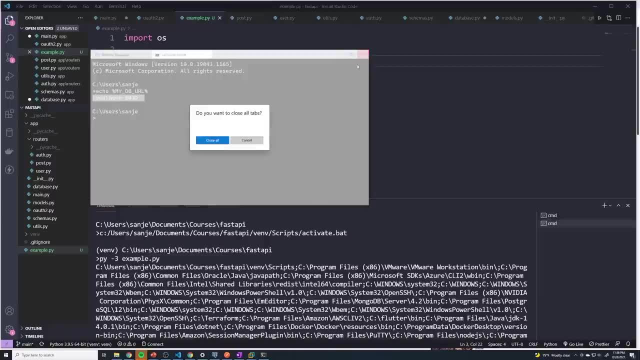 terminals and open up a brand new one. It's kind of annoying, But that's just the way it works. Now, on top of that, there's an even bigger issue- And I think this is exclusive to Windows- And that is that VS code the terminals. here it's: whenever you set a new environment variable, they never 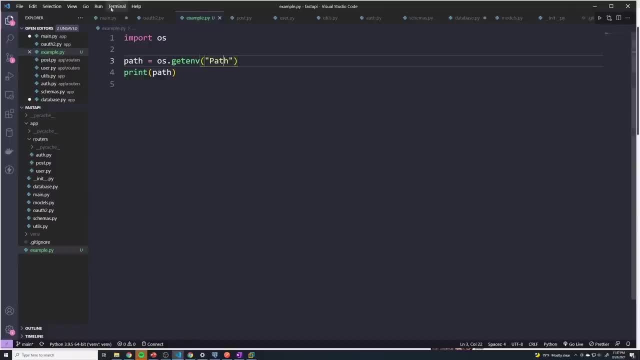 have access to it So you could try deleting all of these terminals and then creating a new terminal And then accessing the new environment variable of my DV underscore URL. And if I try to, I try to access, if I try to run this code, you'll see that it just says none. And if I just tried to run the 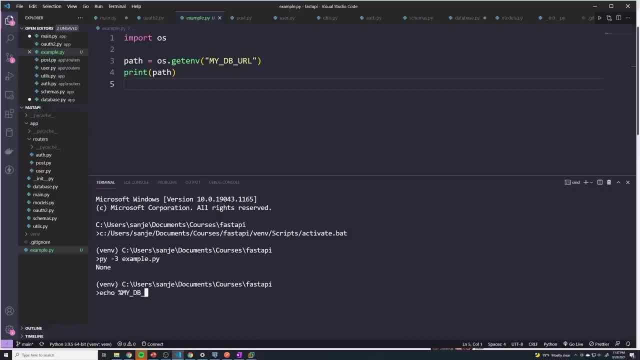 same echo command here you'll see that it just spits it out So it's not able to read that And to read it And it's. it's a little bit of an annoying issue with VS code and windows you have. 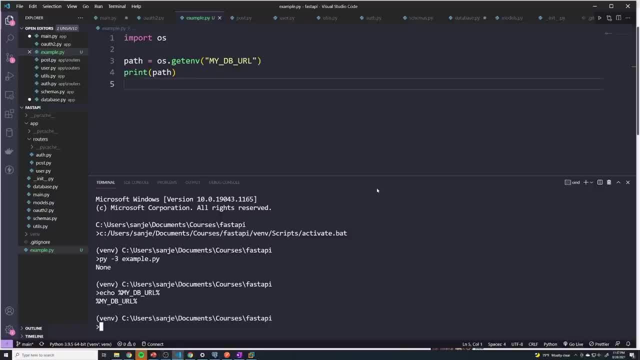 to close out every single VS code window that you have and and then reopen them And sometimes even then that doesn't fix the issue. So know that this is just kind of a limitation with windows, But ultimately don't worry too much about that, Because you're going to see that, especially in a 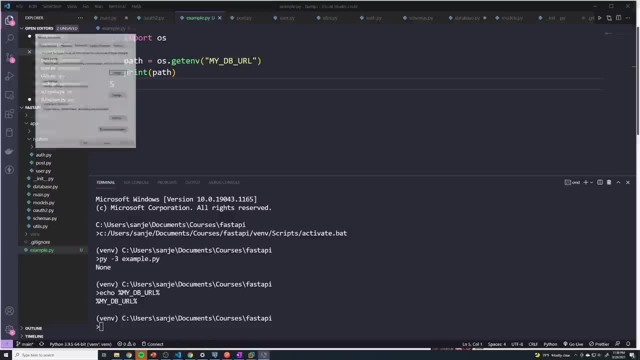 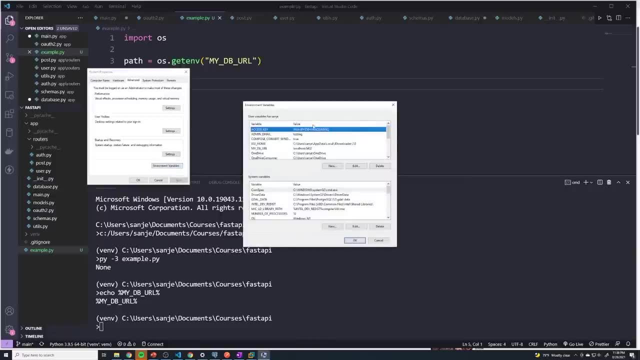 development environment. going into and actually setting all of these variables yourself is unnecessary, right? I don't want to have to go in and set one for my database IP, my database port, as well as my secret key, my password, my username. that's just too many to manage yourself. 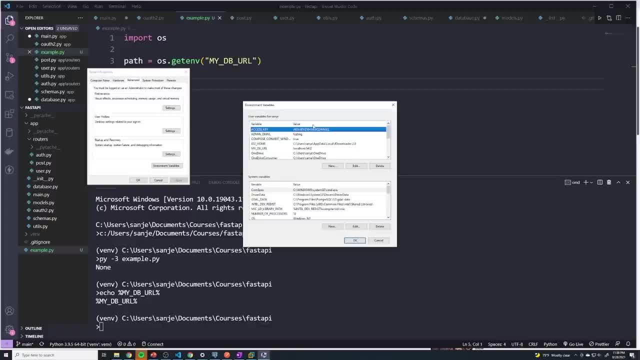 And you'll see that more complex applications could have 10- 2030- environment variables that need to be set. So, instead of going into your system and actually changing it, I'm going to show you guys in the next video. I'm going to show you guys how we can get around this by using 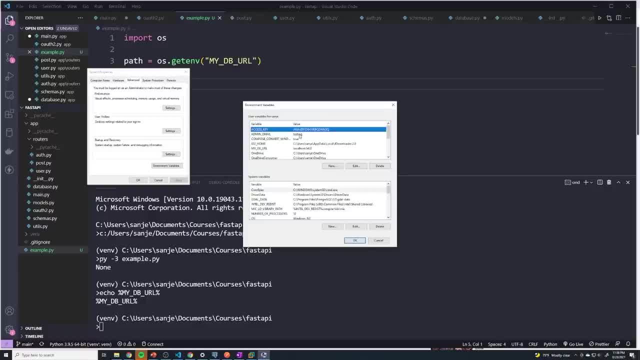 what's referred to as an environment file, And so you don't actually need to worry about the limitations around it. You don't need to worry about the limitations around it. You don't need to worry about the limitations around it. You don't need to worry about the limitations around it. 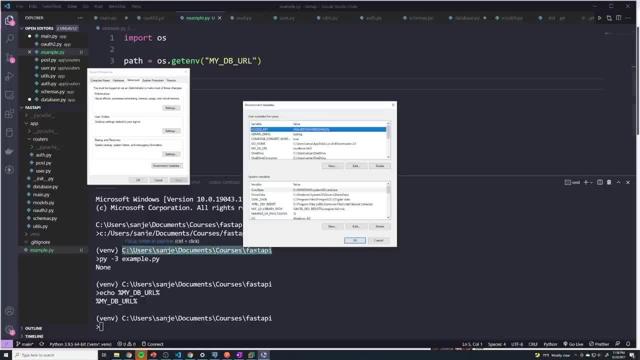 Because we're never actually going to set our own environment variables on our local machine, especially in our development machine, because it's just too slow of a process And it makes things unnecessarily difficult to troubleshoot. So, before we wrap things up, if you want to delete, 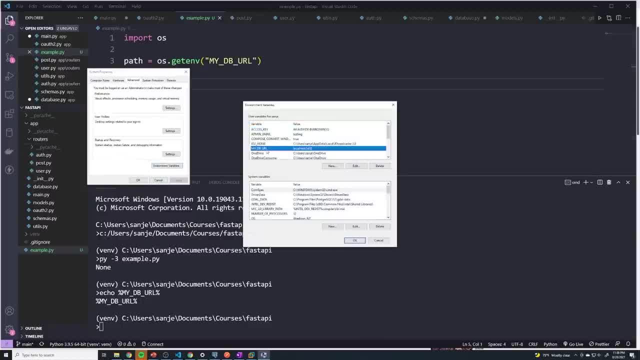 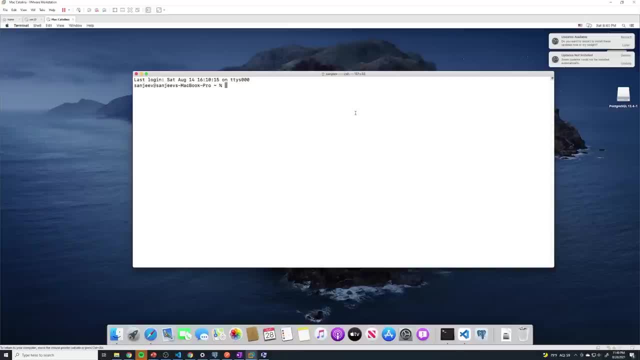 that environment variable. feel free to do that, which we can just go here And I can just select that and then hit delete And let me get. let me show you guys how to do this on a Mac, To set an environment variable on a Mac machine, the command that we run in the terminal. there isn't a GUI. 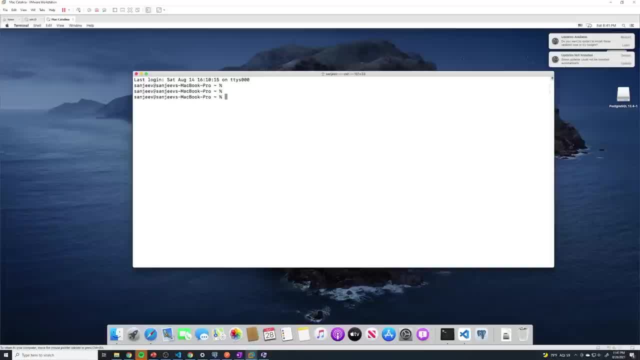 kind of like in Windows. We actually have to use a terminal, which I actually prefer. what we do is we just type in the command export And then we provide the name of the or the name of the variable or the key. So I'll say my underscore DB, underscore URL, then we say equals And then we just provide the text. 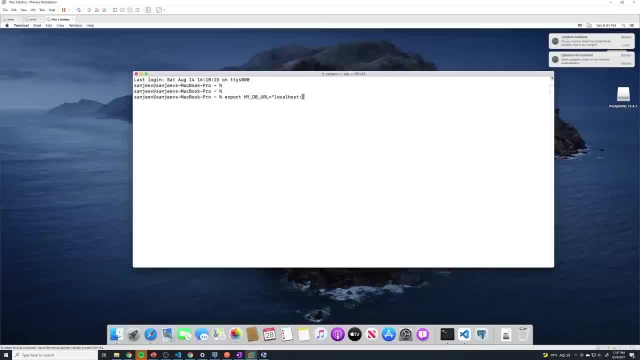 the value. So in this case, maybe this is localhost on 5432.. All right, and then to actually read the environment variables that have been set, you type in print and V, And here we can take a look at all the environment variables. most of these have been. 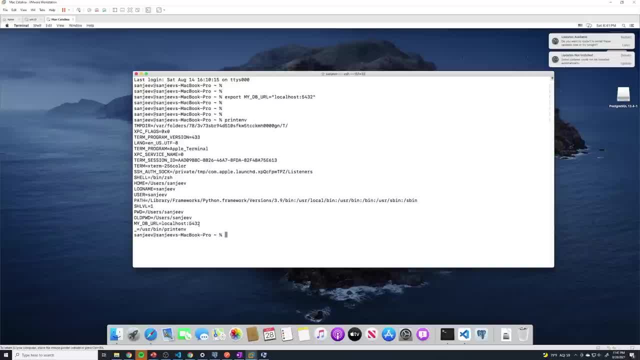 set by the machine itself And you'll see that nowhere in here. do we see? Well, actually we do see my DB URL right here. However, just like I said, in Windows, sometimes you know, depending on the terminal using and a few other things, sometimes you actually have. 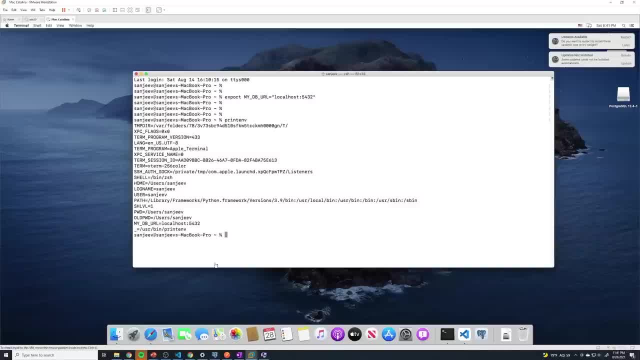 to close out this terminal and open up a new one to actually get the new environment variable. But here we can just access it By typing echo And then we could just say dollar, my underscore DB, underscore URL, And you can see it prints it. 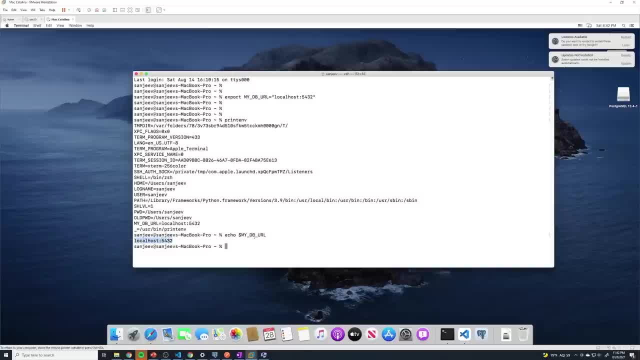 out And then within Python, just like we did on the Windows machine. accessing it is the same exact way. it shouldn't matter depend, shouldn't matter which operating system you're on. It's the same exact thing from your code's perspective. With any project, there's going to be a certain 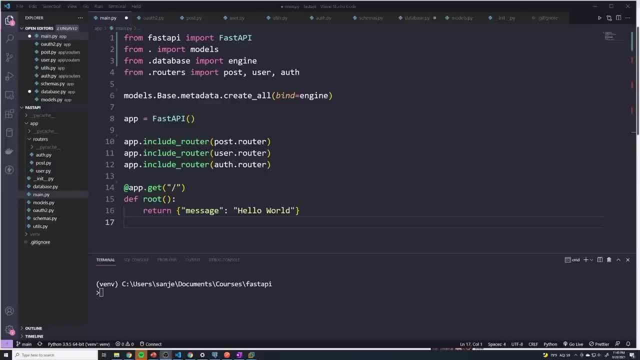 number of environment variables And, as I said, as your project grows, you're going to have more and more of them, And one of the issues that you can run into is that you could potentially forget to set one of them, either on your development environment or your production environment. 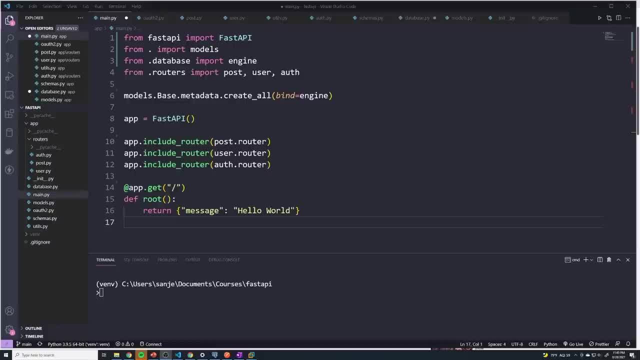 And it's probably going to cause your application to crash, And so what would be good is to perform some sort of validation to ensure that all of the right environment variables have been set for your application to actually run properly. And on top of that, it's important to understand that when 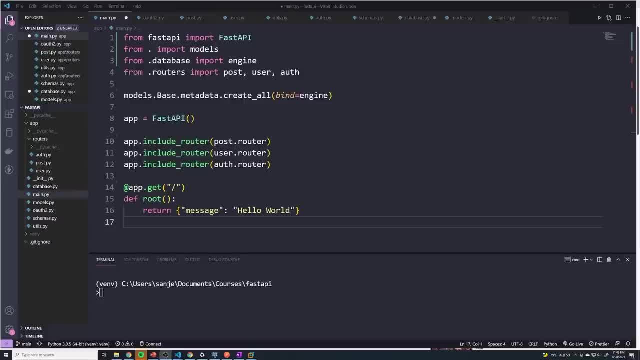 you read an environment variable, it's always going to come out as a string, Which which is fine, but it just means that you have to do all of the validation in code. So if you're setting an environment variable for your, you know your access token expire minutes. 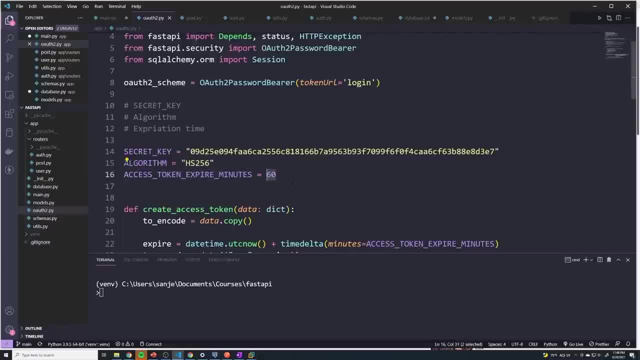 right, we needed this to be an int, not a string, But when we read the environment variable, it's going to come out as a string, So we have to convert this to an integer. So, when it comes to verifying that all of the properties are set, as well as performing validation, 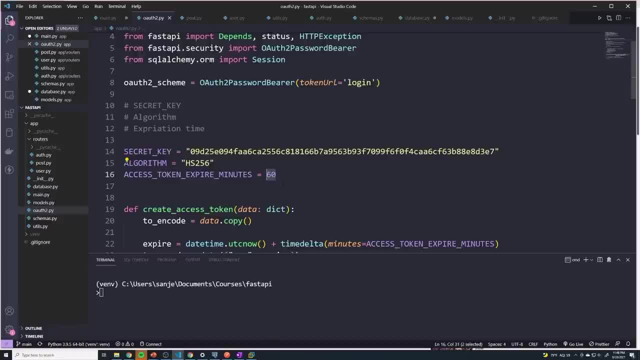 we might have already kind of addressed this issue with a different part of our application. Right, And that's our schemas. right, We do the same thing with all of the data we send in the body by using pydantic to perform all that. 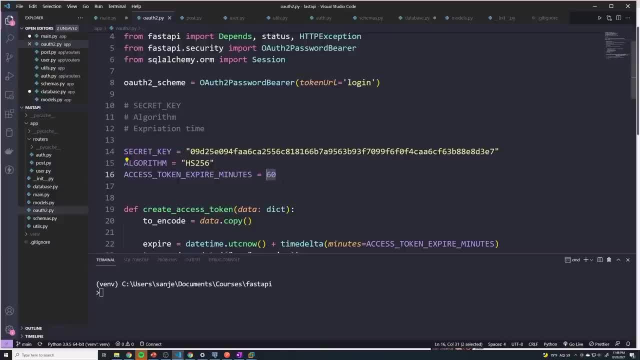 verification to make sure that every single property that we need is there, And to also perform all of the typecasting. So if we set it something to be an integer, it'll automatically convert it and validate it. that is a valid integer, And what's great about pydantic is 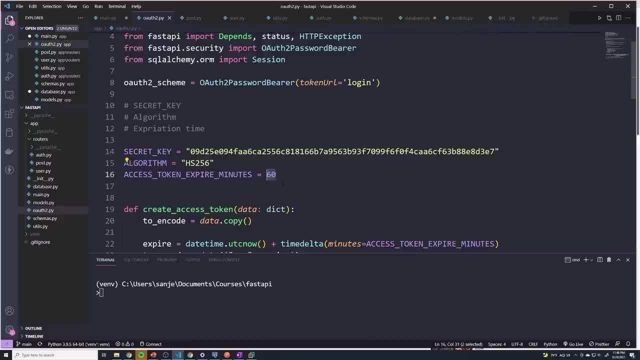 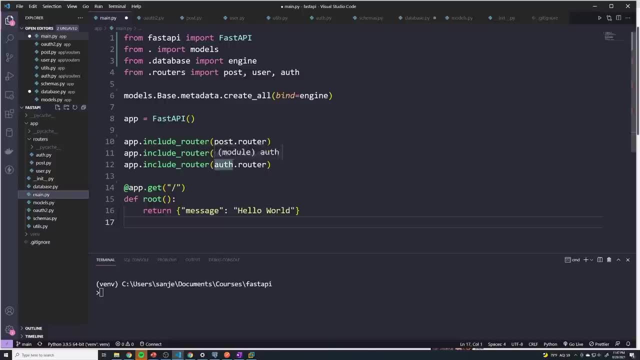 we can actually use pydantic to perform all of that validation for our environment variables, And let's see how we can actually do that. So I'm going to go to mainpy And, as an example, I'm going to go to my environment variables And I'm going to go to my environment variables. 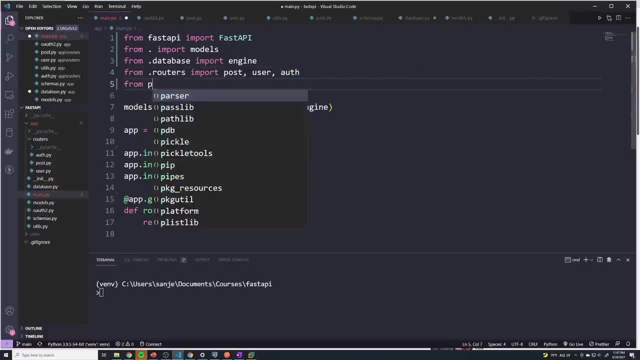 And, as an example, I'm just going to import from the pydantic library something called base settings And so, just like with, you know, any other pydantic model, right, we can set up a class And I'm going to call this settings, And this is going to extend base settings. 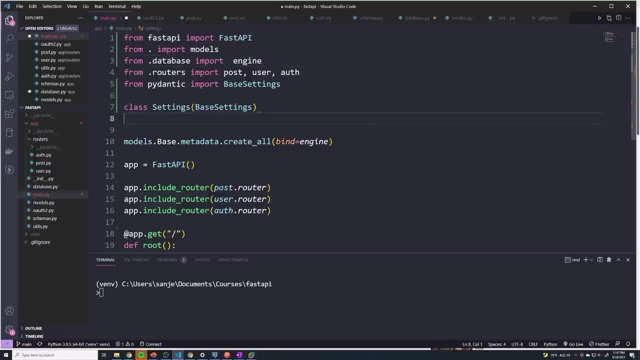 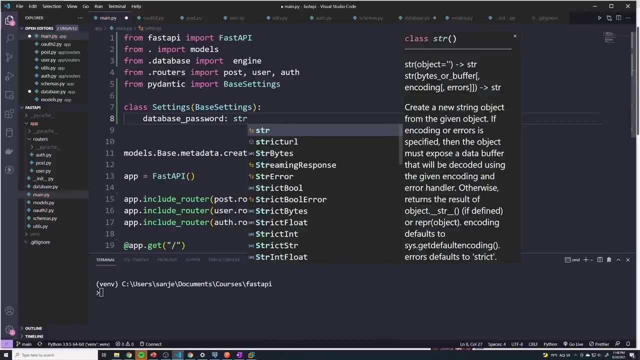 And I didn't mean to accidentally import base, And here we can basically just provide a list of all of the environment variables that we need set as properties on the class itself. And so you know, maybe I need something called database underscore password, And this needs to be a type string And we can even give it a default value. 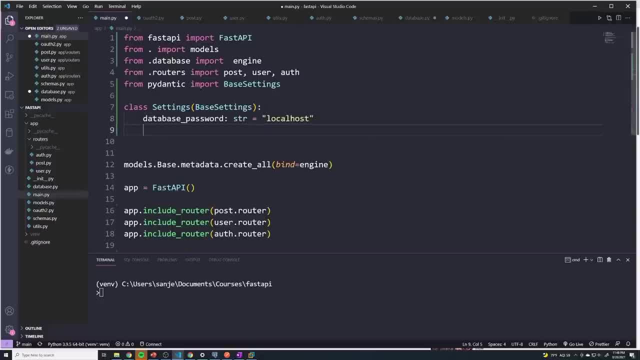 which is local host, And then maybe I need a database username, which is going to be string, and we can give it once again a default password. we don't actually have to get a default value, But if you want to, you can, and I'll say this is going to be Postgres. 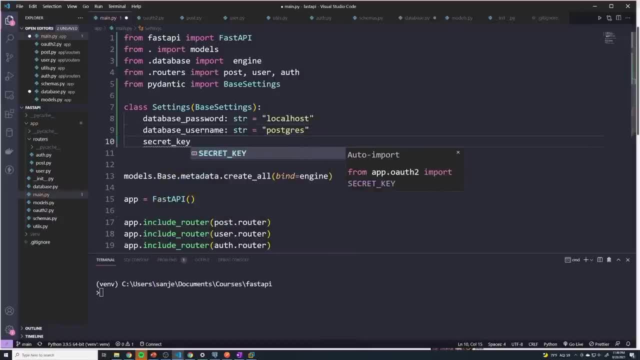 And then maybe we want the secret key, And this is once again going to be a type string and we can just give it, you know, some arbitrary default And let's say these are the only environment variables that we need for our 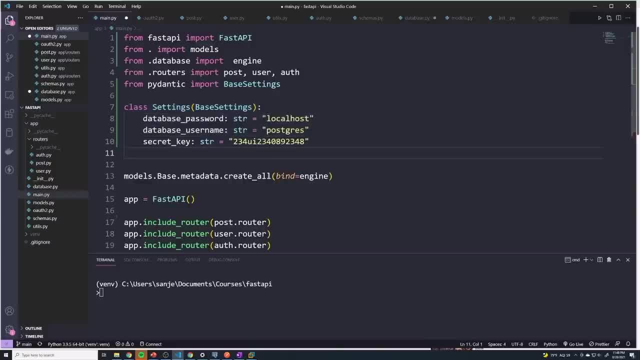 application to run. By setting it like this, it's going to automatically perform all of those variables And then we can set the validation for us to ensure that all of these have been set. And an important thing to understand is that when you set environment variables, you know if we just quickly 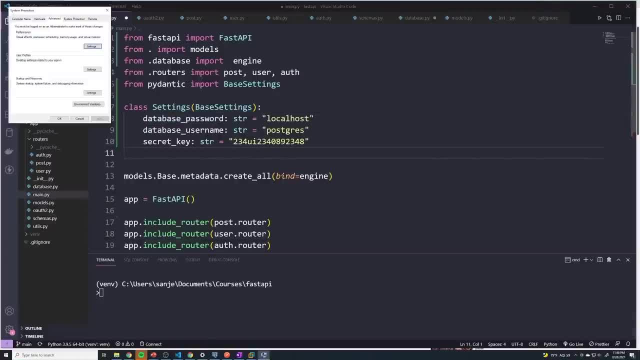 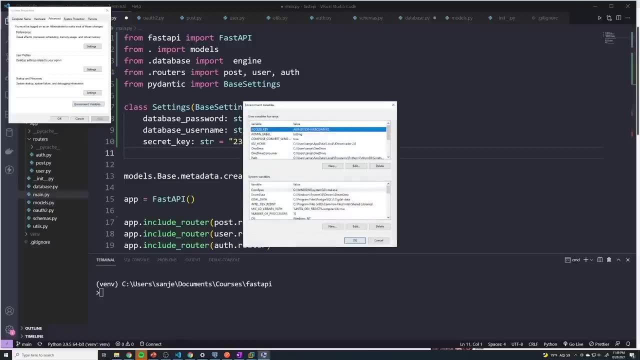 go back to the environment variables on my machine. Normally best practice for environment variables is to do all caps with underscores. right, It doesn't have to be all caps, But this is just kind of standard convention. you can see, I've got some. 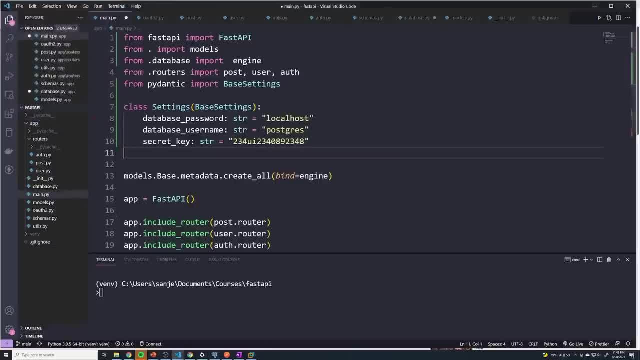 that aren't like that. But in general you want to do it all caps- And you can see, here we can do it all in lowercase. So pydantic will automatically handle all of this from a case insensitive perspective. So it doesn't matter if you capitalize this or lowercase everything, it'll. 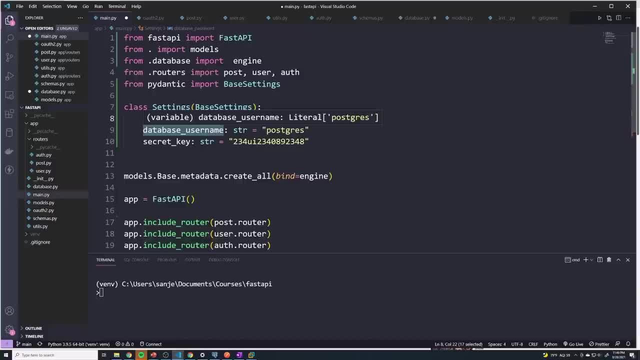 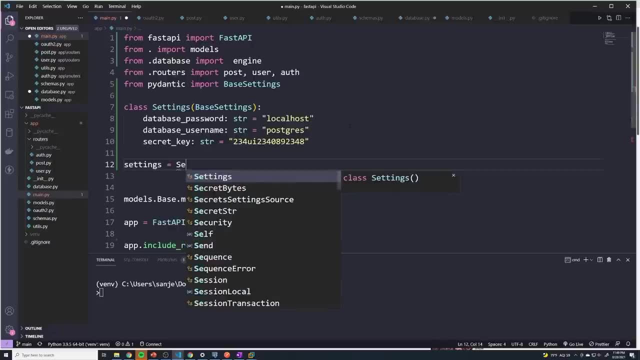 take all of your environment variables and it'll convert it to lowercase. just to simplify everything, then we create a variable called settings equals, and then we say settings. So right here, all we're doing is we're creating an instance of the settings class, And so at this. 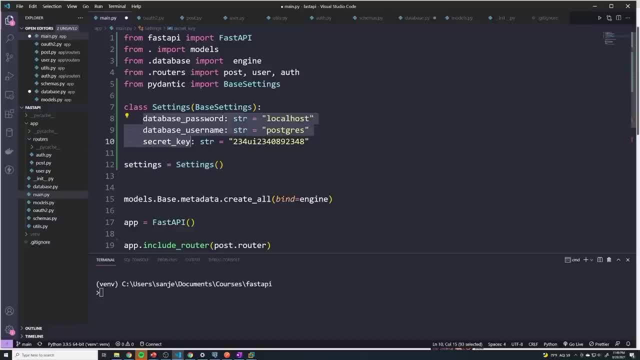 point. it will read all of these environment variables And once again it'll look for them from a case insensitive perspective, So it doesn't matter if they're capitalized or not. And then it's going to, and then it's going to perform all of the validation. it's going to ensure that they're. 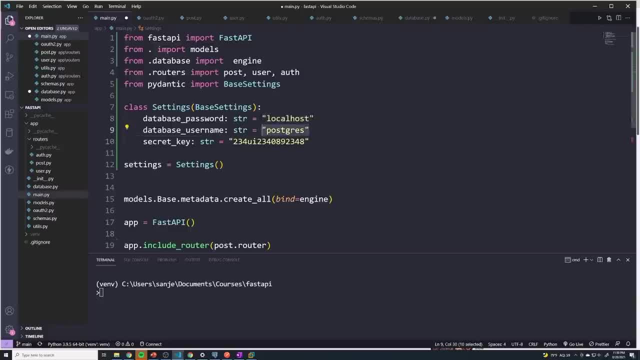 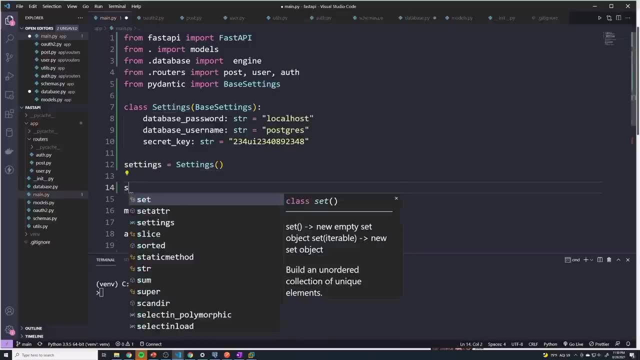 properly a string and and so on, And then finally it's going to store it in a variable called settings. So then we can access all of these variables by just saying settings, dot and then the name of the property. So if I want to get the database password, I just do settings dot- database. 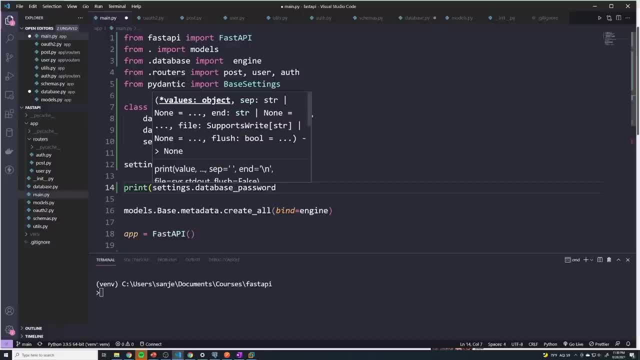 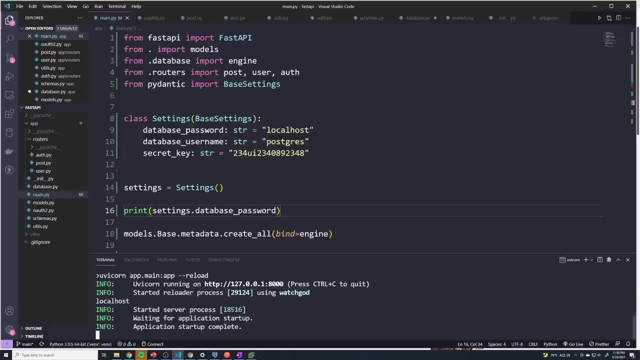 password. Okay, Oh, I just want to get this right Now. I'm going to try this out And I'll just start my application Right And you can see that it printed out local host And if I want to grab, maybe the 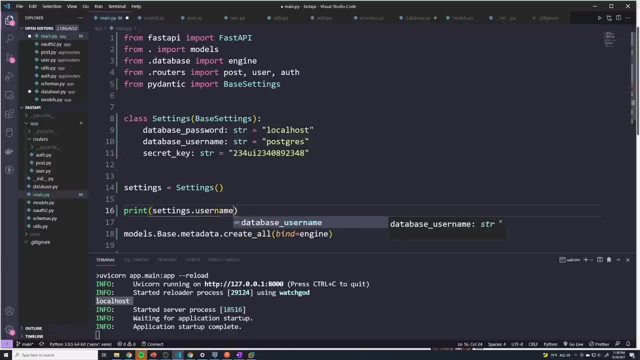 username. I just say username. actually side should be database, underscore username And you nue t see it prints out Postgres, which is the default values, because I haven't actually set my system environment variables and I'm all just going to just台. 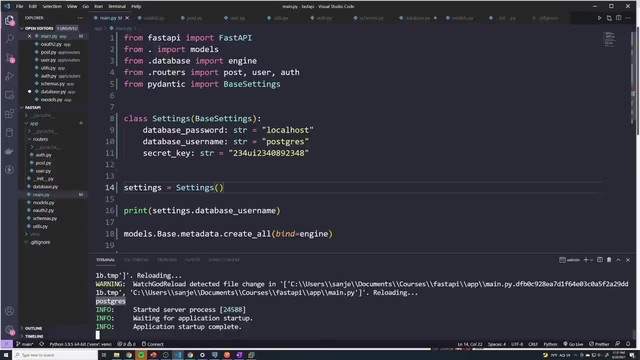 divai Michelle Takachori voice Tell Google: Billy, You specialised. you're welcome to variables to be any of these values. So it's going to use the default one And, like I said, we're going to run into that Windows issue where I can't exactly update it without closing. 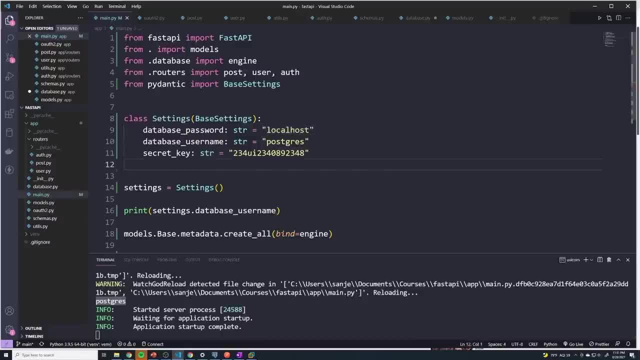 everything. So I'm not going to bother doing that. But what I will do, just to show you how this validation works, is: let's remove this, Let's say there's no default password, And so if there's no default password, then you know it's first going to check my system, my, my system. 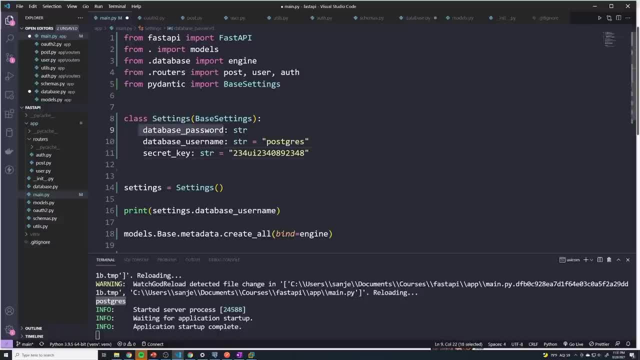 or user environment variables to see if there's something called database password And since I didn't provide a default one, if there is no environment variable with that name, it's going to throw an error, because the whole point of this is to validate that all of the environment. 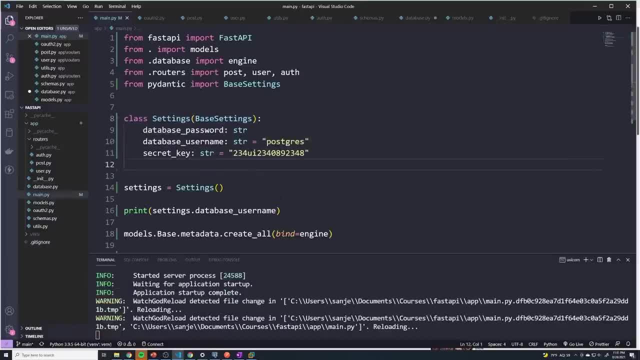 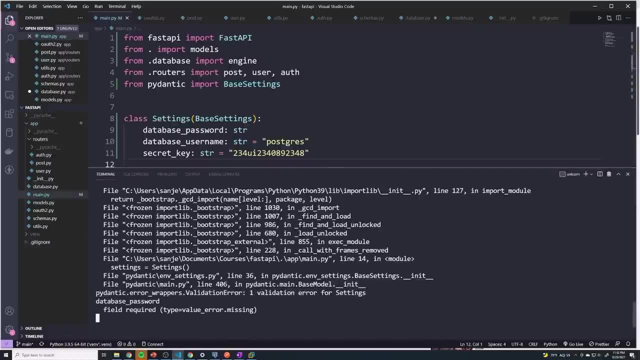 variables that we have are configured here, And so after I save it, if we take a look at this, you can see that we get one validation error for settings, So settings database password, and we can see that it's missing Right, And so having that quick check it makes our life so. 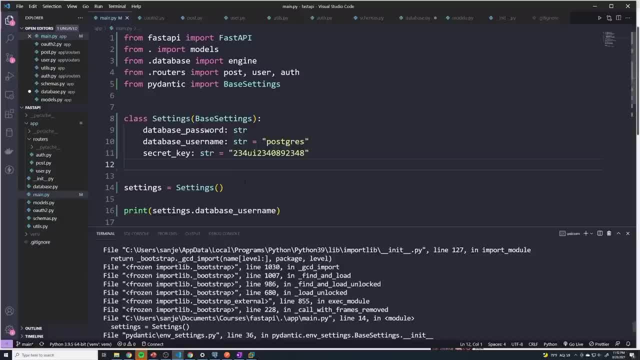 much easier so that we don't have to figure out you know which environment variable is is missing, which one's not, because, like I said, you could have 10, 2030, 40 of them. there's gonna be a lot of them And 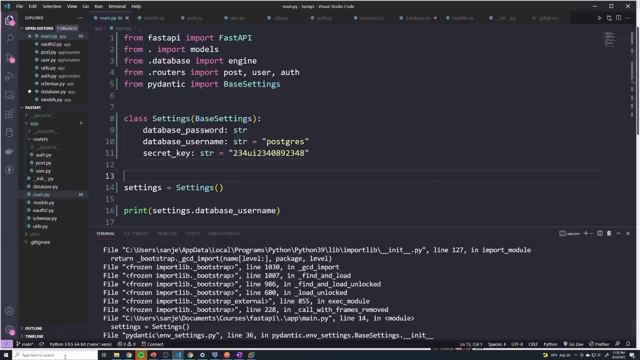 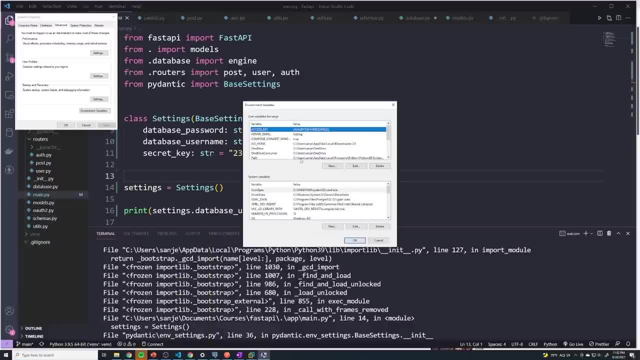 managing them does become a little bit of a challenge. Now one quick thing, you know. let's say, I go to my environment variables once more And I've got something called path, right, So path is you know something? the path to a specific directory. And what I'm going to do is I'm going 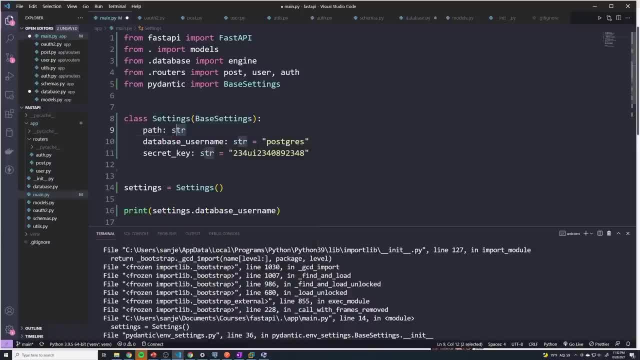 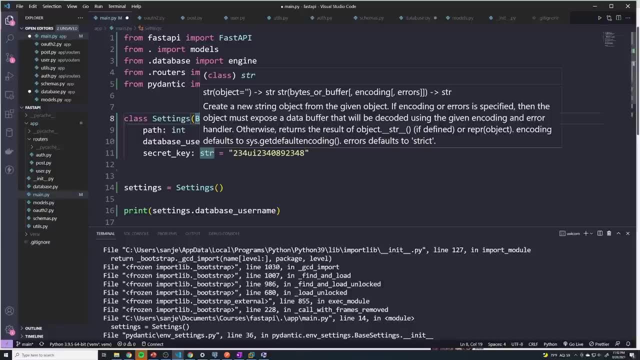 to say: I want to access the path, But we're going to say that this needs to be of type int. So pydentic is going to form some validation, it's going to read it and every environment variable is always read as a. 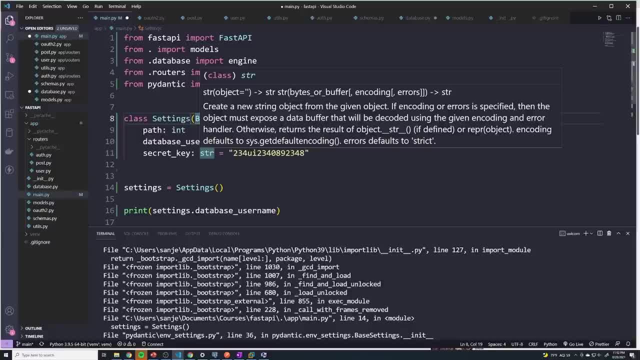 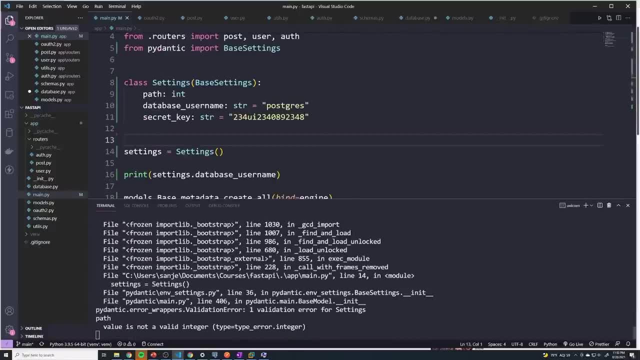 string And then it's going to try to typecast it into an int And if it fails, it's going to throw an error, And so, since this is clearly not a integer, it should throw an error. So let's try this out And we can see that value is not a valid integer. Now for all of the settings in the. 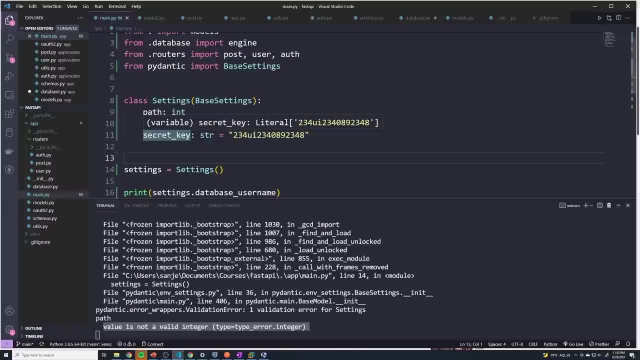 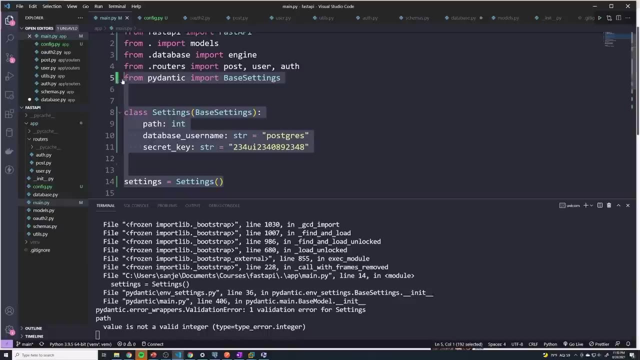 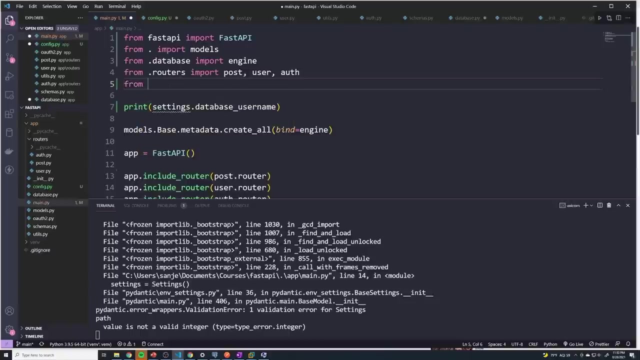 environment variables. I usually like to create a separate file to hold all of this information. So under app I'm going to create a new file called config dot p y And I'm going to move all of that code into that file And then in our main dot p y file I'll just import from dot config. import. 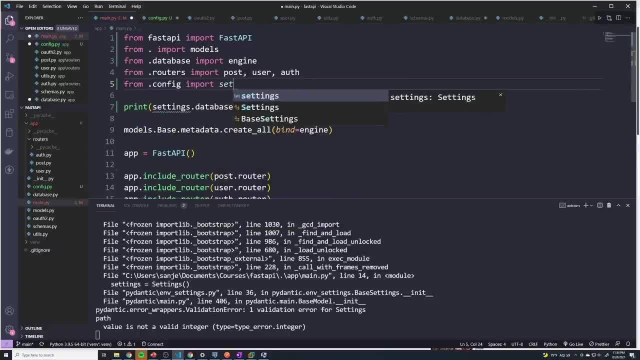 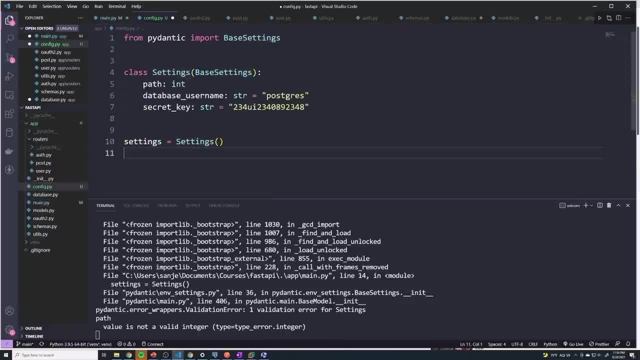 settings Right. So ultimately, we're just importing that final class, the instance of the class that we created- Right, And so, once again, it's able to perform the validation. it's going to report an error with the path variable. 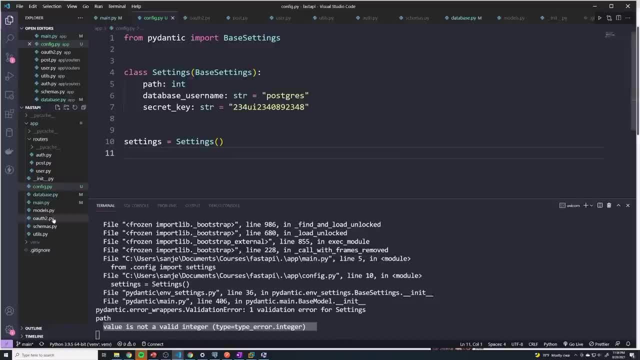 Alright, so having it in its own file is going to make things a little bit easier, because then we could just go to the configpy file And we'll know exactly you know where to look for all of our environment variables and all the configs related to our application. 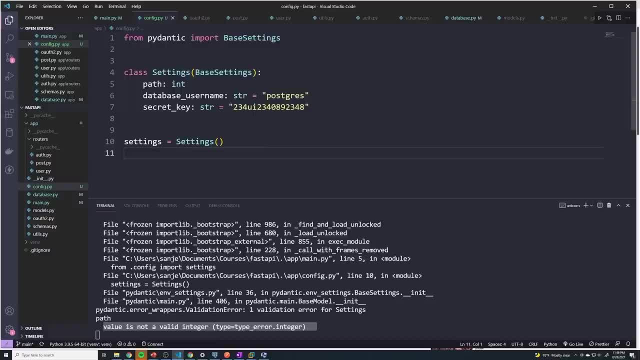 The last thing I want to do is let's go ahead and actually figure out what environment variables we want to use, moving forward, and actually set this up. So we're going to clear out all of these And I'm going to create one for all of the database related stuff. So database underscore. 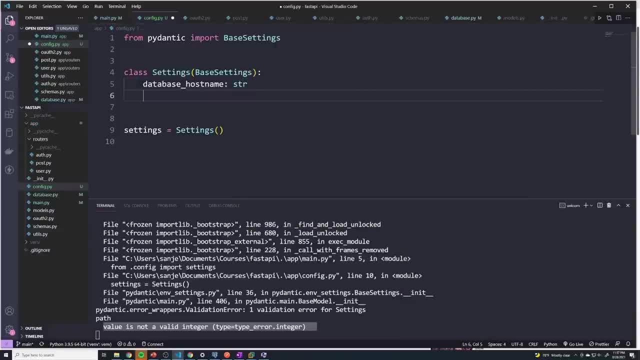 hostname is going to be a string by default. we're going to have database underscore port- Once again a string. we'll have a database password And then we'll have a database underscore name. So that's the database within Postgres that we're connecting to. 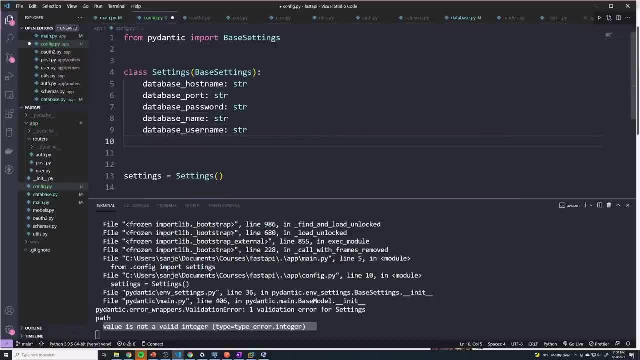 We'll need a username. all of these will be strings And you may be wondering why the port is set to a string. But the reason why it's going to be set to a string is because, if we actually take a look at our database connection, 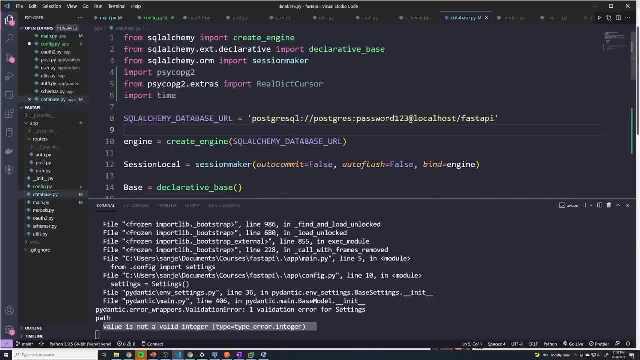 it just goes into a URL, So we don't actually ever need to have it be an int. I guess you could make sure that it's a valid port number and then convert it back to a string, But that seems a little unnecessary at that point. Then there's a secret key for 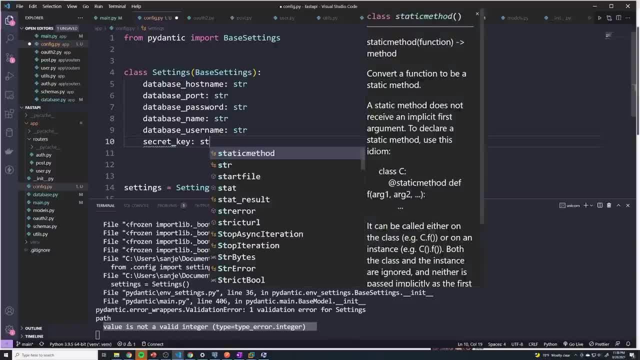 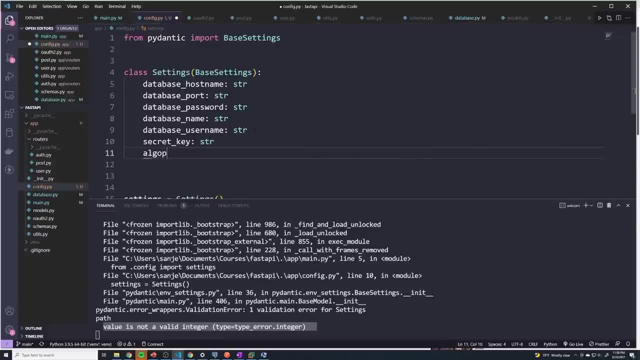 or you know our JSON web tokens. We've got the algorithm for signing our token And then we have the access token expire underscore minutes, which is going to be an int. All right, And if we save all of this, we should get a whole bunch of errors, And that's okay. 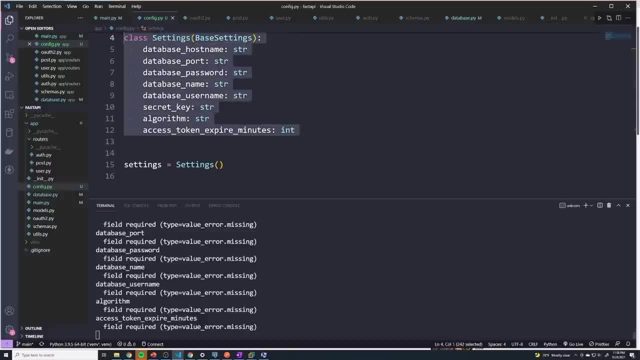 because none of these have been set. So at this point you could technically- you know whether you're on a Windows or Mac- set these on your machine and get everything to work. But, like I said, that is an unacceptable thing to do because that's a lot of work And we want to simplify. 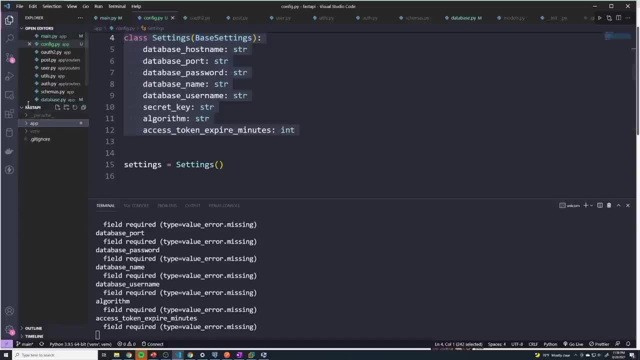 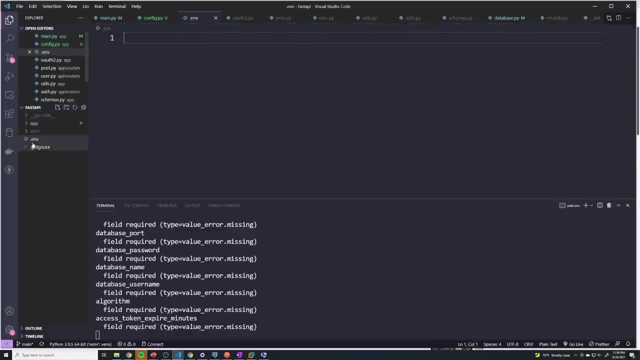 things. So what we can actually do is, within our fast API directory, we're going to create a new file called dot env. So this is kind of standard convention. But this file- and don't forget the dot- this file is going to contain all of our environment variables, So we can set it much. 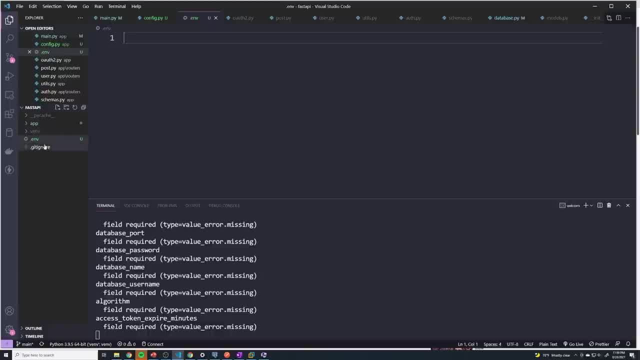 easier just by having a file do all of the work. Now, in production, you're not going to use this in production, you're going to actually set it on your machine, But in development it's perfectly okay to just set everything in here, And so what we're going to do is we're going to take all of 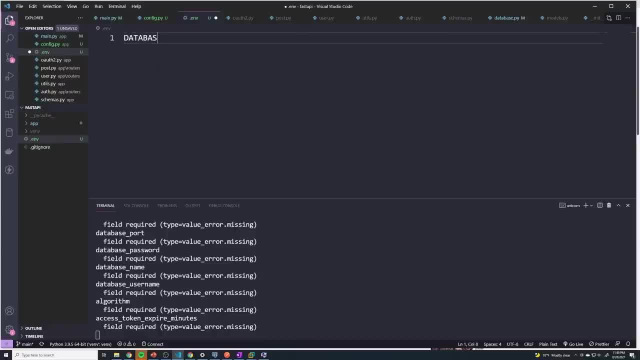 those environment variables that we defined and we're going to provide values, And so, like I said, in real life you generally want to capitalize everything, But luckily, Pydantic automatically looks at everything from a case insensitive perspective, And so our database right now is: 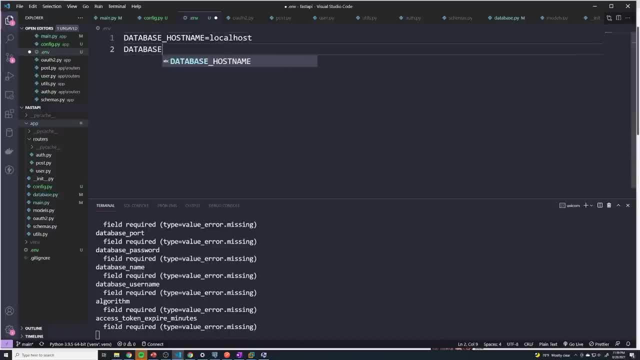 running on localhost, So we can just say localhost. Our database port is going to be 5432.. The password that's going to be whatever you chose to use as your password. It's gonna be password 123. And we've got our database name. 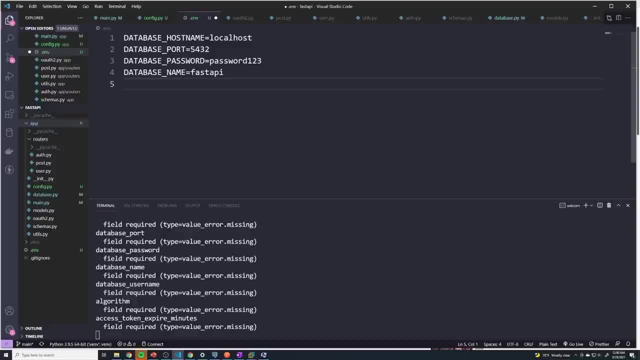 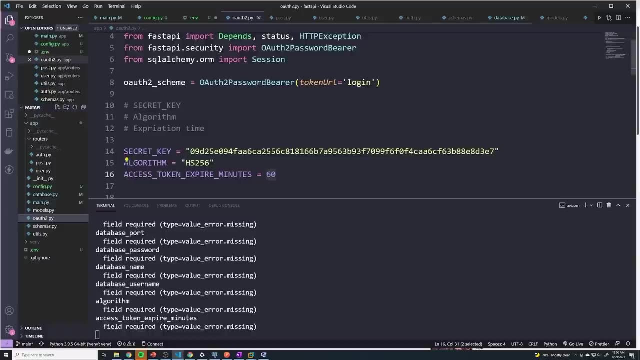 Mine happens to be fast API, but yours is going to be something different, probably The username. I'm guessing everyone's probably going to be using the default Postgres, The secret key. I'm just going to grab whatever I used in my file, So I'll just grab this. 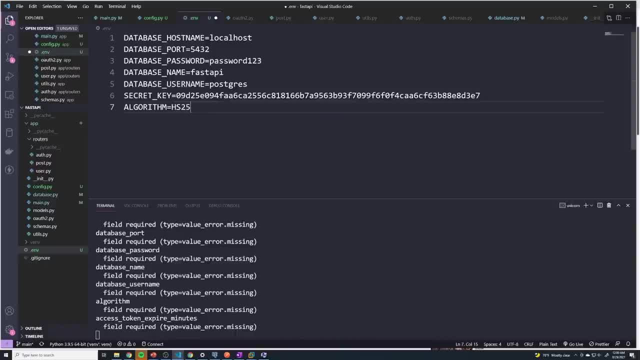 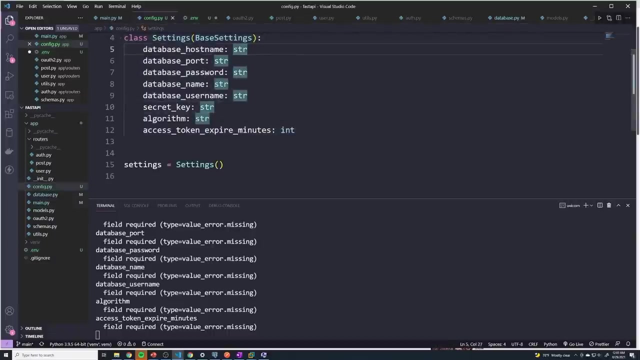 The algorithm is going to be HS 256. And then the access token expiration time is going to be set to 30.. So we've got all the values set here. And one thing to note: I didn't provide any default values and you could 100% go ahead and add default values into yours if you want to, but I'm going to leave. 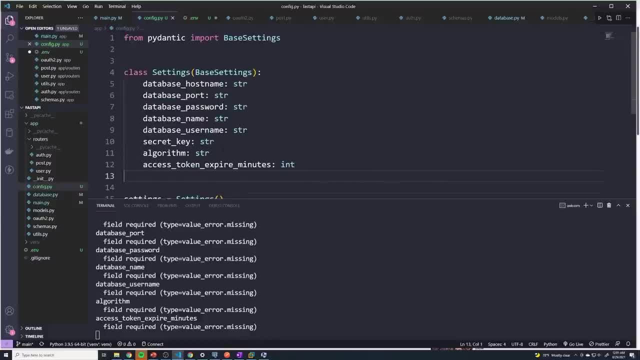 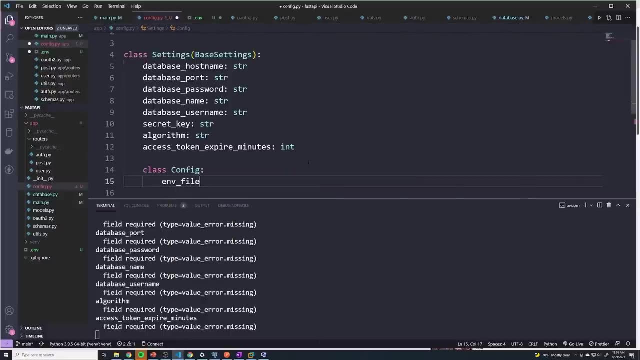 them as such. And now we have to tell Pydantic to actually import it from our env file, And the way to do that is inside this class. we just say class config And we say env- underscore file, and then the path to our specific file. So we say dot- env. So we'll save this And I forgot to. 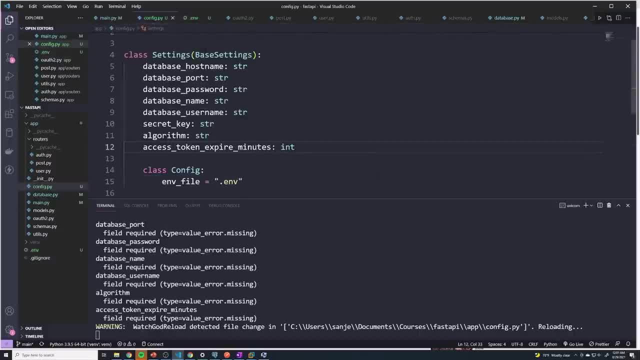 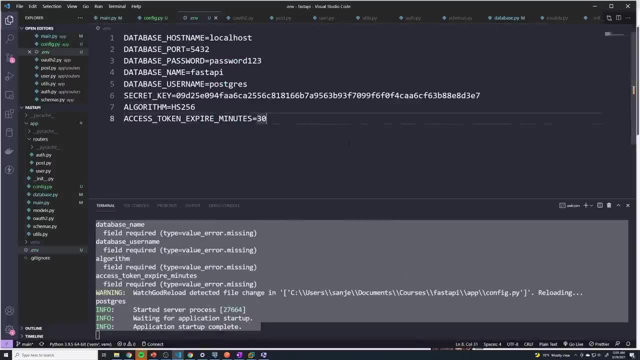 save my env file And then I'm going to run this again And our application should start up with zero issues. And so hopefully you guys see how easy it is to work with environment variables, especially when you're allowed to set it on a file. 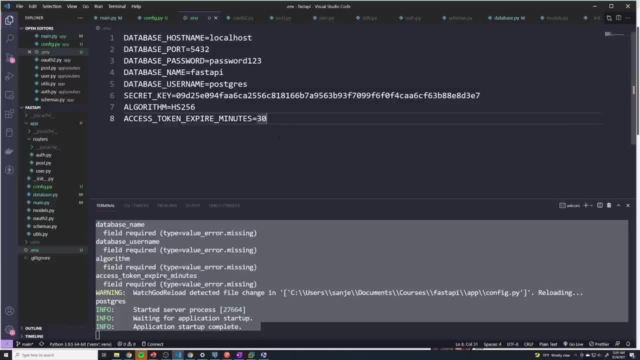 so that we don't have to worry about setting it either in the terminal or, you know, on a Windows machine, having to go through the GUI to do that. But one thing to keep in mind is that you never want to check this ENV file into Git, right, Because this has all the credentials for your 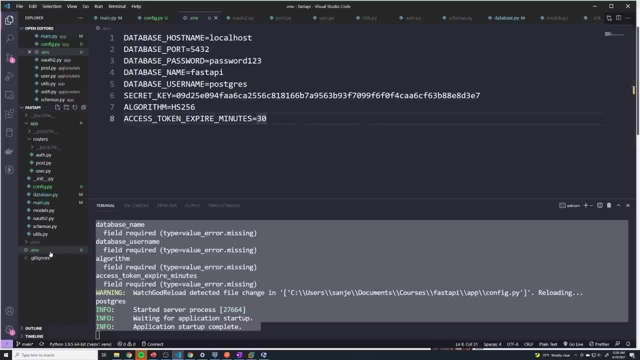 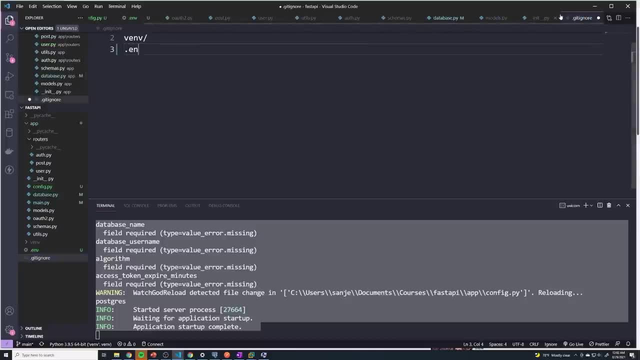 development environment. Maybe you don't want those to get out And there's no need to ever check it into Git. So if you create a git ignore file, so, which is dot git ignore, you want to make sure that you put in dot ENV And we'll come back to the git ignore file when we start working. 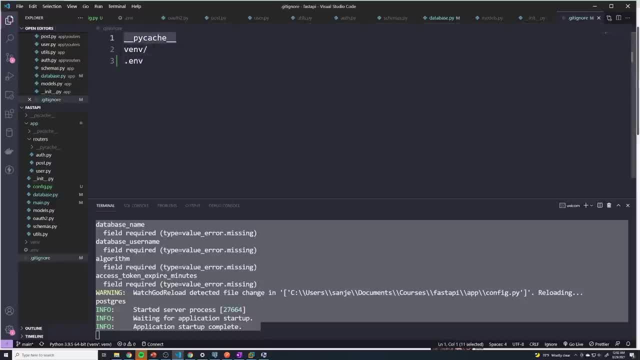 with Git in this course. But you also want to make sure you remove anything with underscore, underscore, PyCache, underscore, underscore, which is all of these, as well as your virtual environment folder. So you want to make sure none of those get checked into Git so they don't get uploaded to. 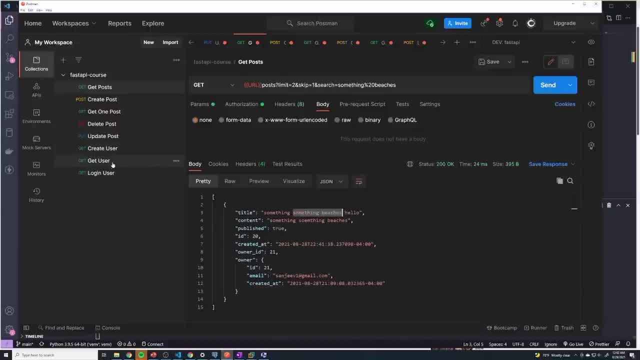 your GitHub repo And just to make sure that everything's working, let's go ahead and just test this out real quick, just to make sure that nothing's broken. And that seems to work. And if we try to get all posts, everything seems to be working. So we have now successfully moved everything over to environment. 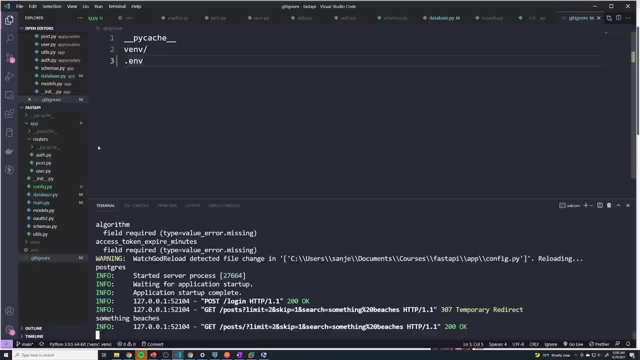 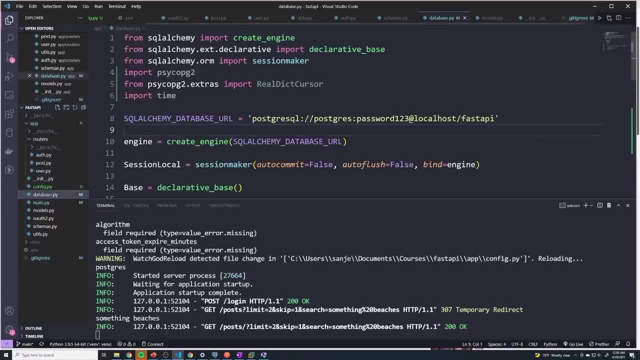 variables And actually sorry, we forgot to do one very important thing. We're not actually using the environment variables right now Because if I actually go to my database you can see that it's still just a hard coded value. So we have to make sure we actually update that to use the 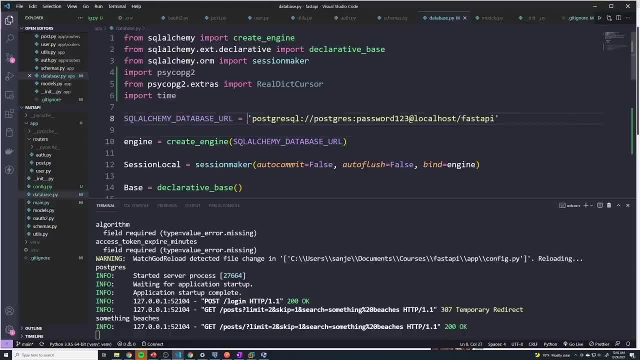 environment variables. So we're going to change this to be an F, an F string, And then here, this is going to be the username, this is the password, this is the host name, and then this is the database name, And then there's also going to be: 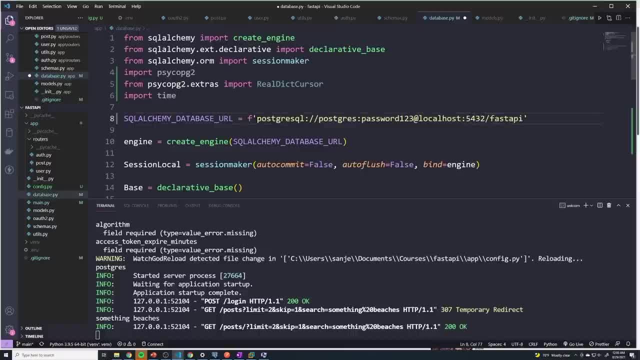 the port number, which would be right here, which is 5432.. I believe that's. Yeah, and that's going to be the port number. So what we have to do is, since we're using an F string, I can just remove this. 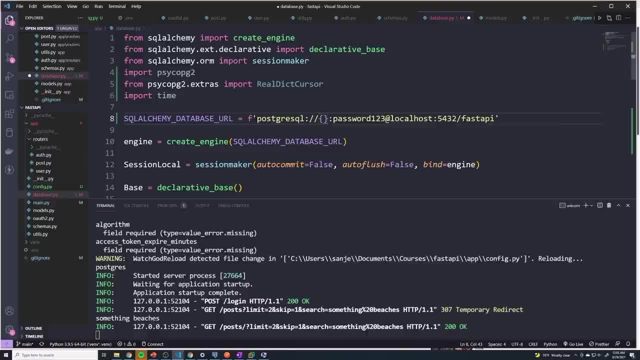 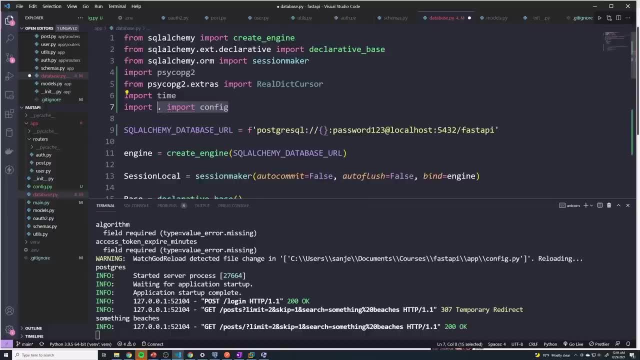 And I can say: well, first of all we have to import our config file. But we have access to it, Or we can do from config Import settings. Just put a dot there And now I can just say settings, dot database, And then we'll grab the. 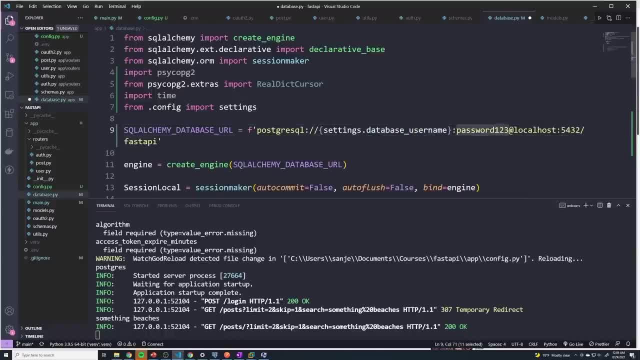 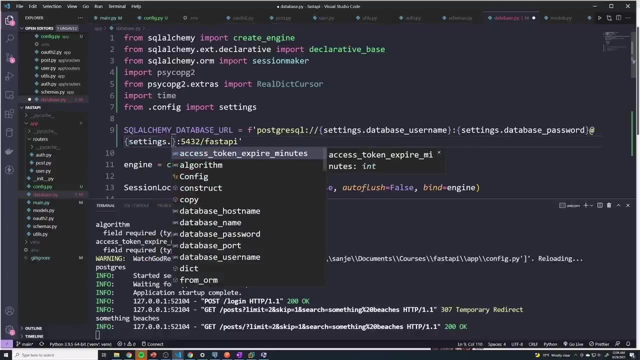 username here And then for the password, I'm going to do the same thing. I'll say settings dot database password And the host name. This is going to be settings dot database host name, And then there's going to be the 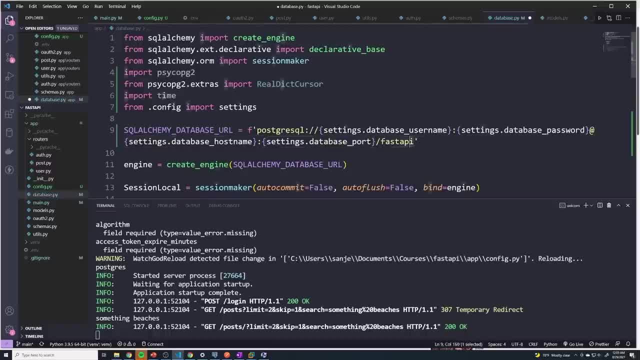 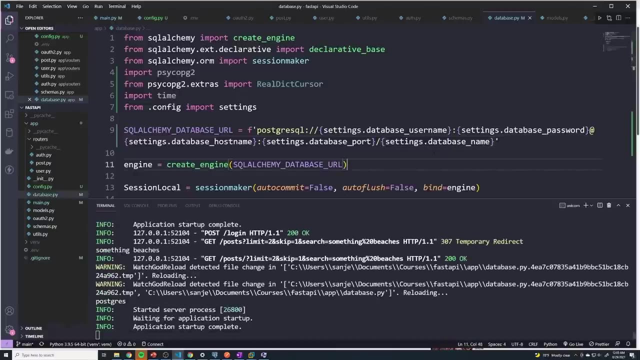 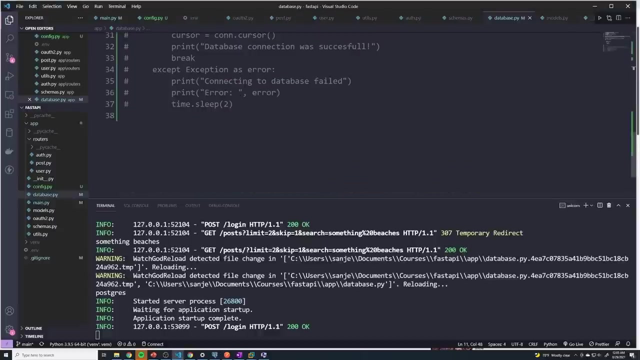 port number And then, finally, we've got the actual database name. I think everything should still work. just to test this part, Let's just quickly log in now. All right, everything still works. So we are access to our database is now working just fine, But there's a few other things. 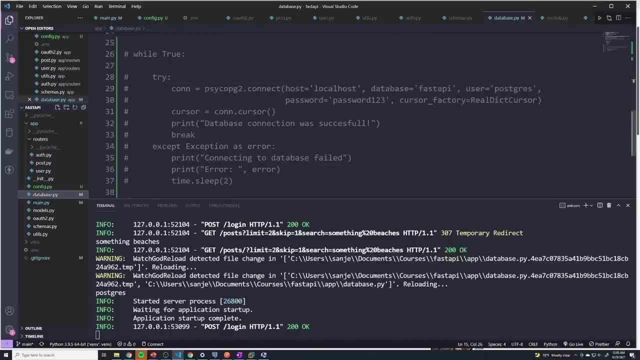 that I want to update And keep in mind. if you're using the Postgres driver to actually connect and make queries, then you would just update it here with the settings dot, whatever. But if we go to our OAuth two, we can Well. first of all, let's import. 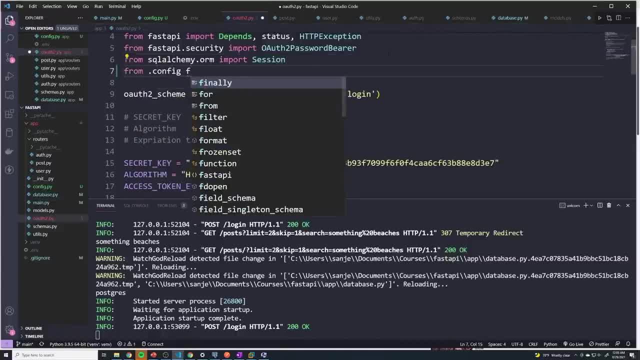 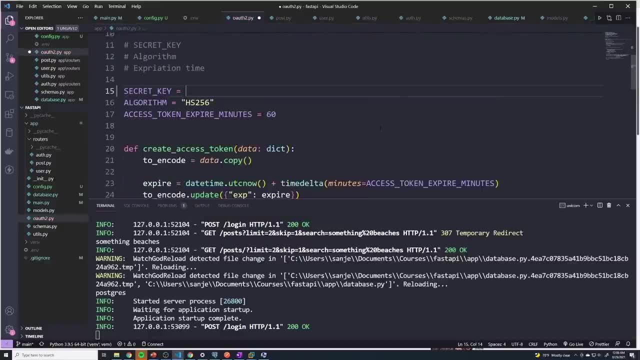 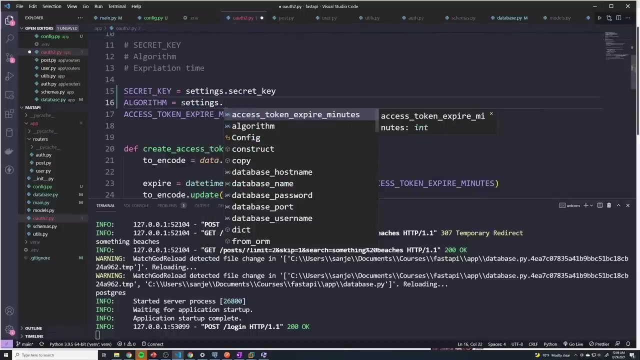 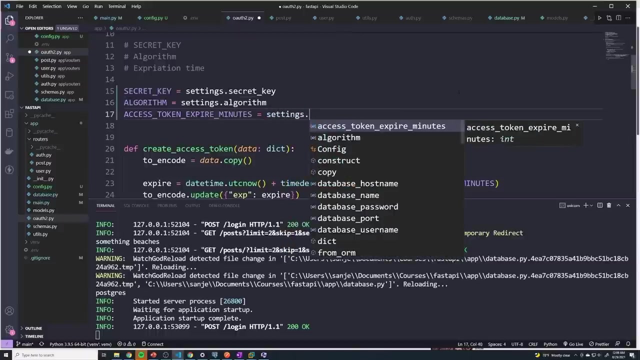 our config And we'll change the secret key. This is going to be settings dot secret key, not schema secret key. The algorithm is going to be settings dot algorithm And then, finally, this is going to be settings dot access token expire minutes. 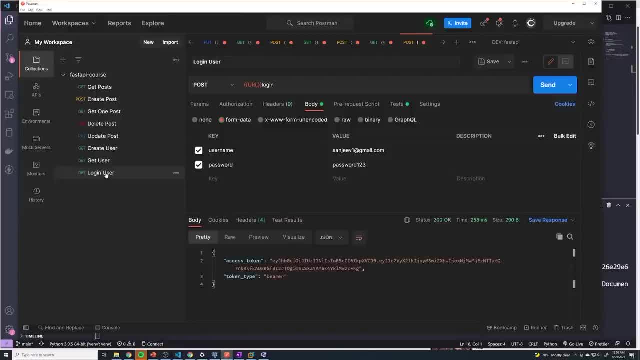 All right, let's reload this. Let's just double check a few things. So let's- well, let's create a new user. All right, we were able to create a user. let's log in that user. We're able to log in, and then let's get posts. And we're able to get posts, And let's just double. 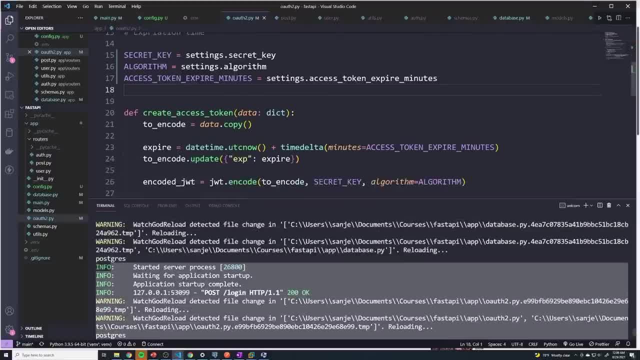 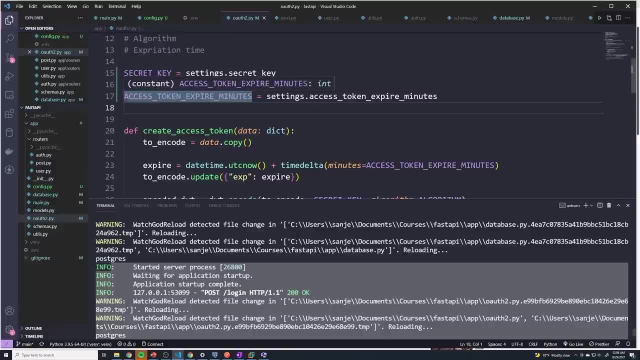 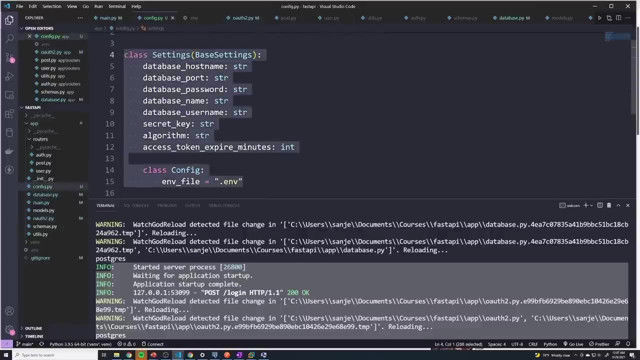 check that there's no errors. So everything looks good. And so now we have successfully migrated all of our code to using environment variables, And so when we move to production we can just, on the machine, set all of these values that we have inside our config dot py file, and it's going to automatically import it. 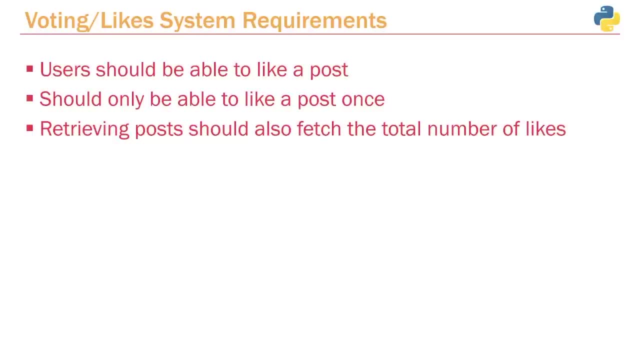 and then update those values wherever we reference them. In any social media type app, there's going to be some sort of voting or likes system. So Facebook has likes, Reddit has upvotes and downvotes, Instagram has likes, Twitter has likes as well, And so we're going to implement a simple like system as well, And we're 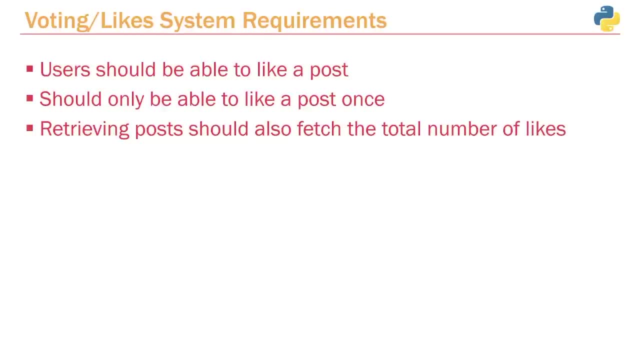 going to quickly go over the requirements for it. So the first thing is: a user should be able to like a post. a user should only be able to like a post once. we shouldn't be able to like a post 10 times and then artificially cause the number of likes for that post to go up. And then finally, 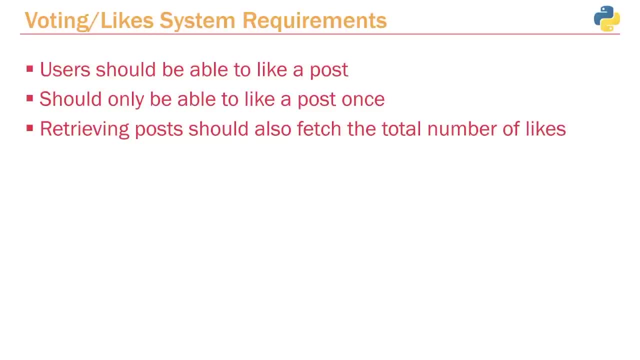 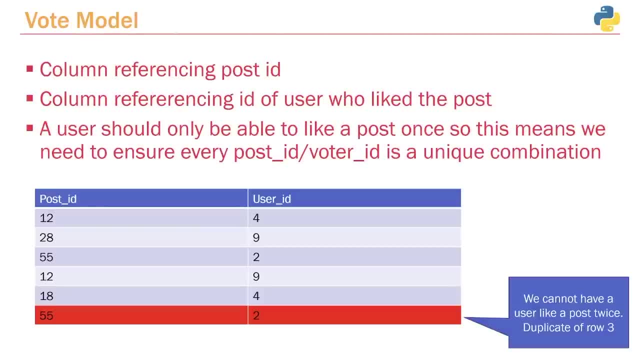 look at the requirements for our voting model, or like model, And so naturally, just like we have a table for users and a table for posts, it makes sense to store the votes in another table, just like we always do. And if you think about the requirements or what we should do for the columns, 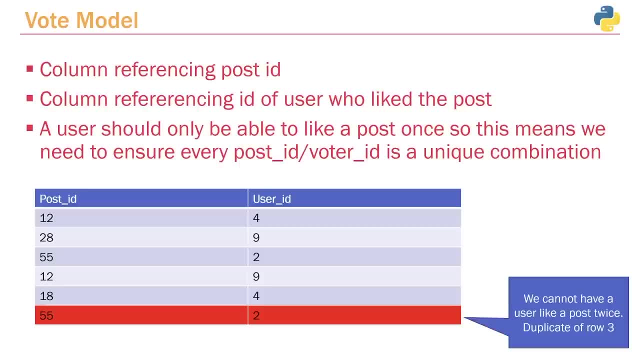 well, we need to have a column that's going to store the ID of the post that we're ultimately going to like, And then we're also going to need a column that references the ID of the user who liked the post. So those are the two absolute minimum number of columns that we need to get our voting system in. 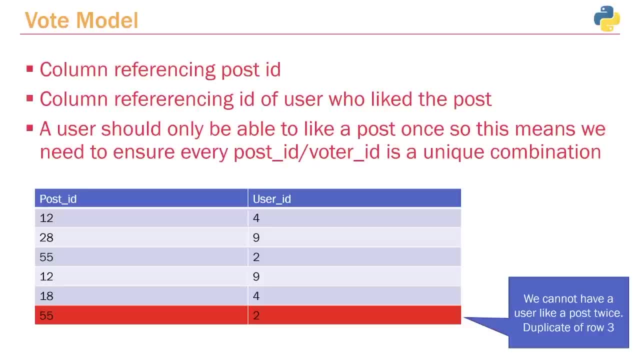 place. Keep in mind, if you wanted to do a, you know, an upvote, downvote type thing like Reddit does, then you might want to have a third column for the direction of your vote. But we're going to keep this nice and simple And it's just going to be a very simple like system. So it's just one. 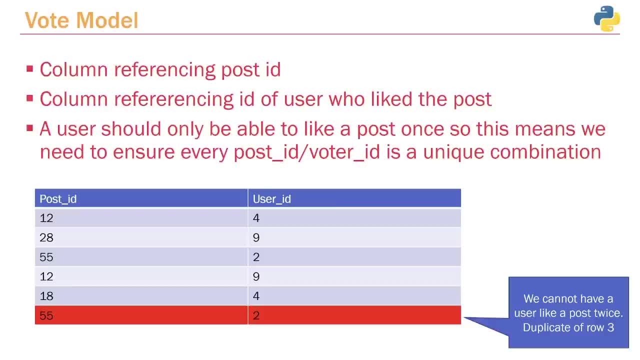 direction. But the most important thing of the vote table is that, since a user should only be able to like a post once, this means that we need to ensure that every entry, every post, should be like a post ID and voter ID is a unique combination. So what do I mean by that? Well, take a look at. 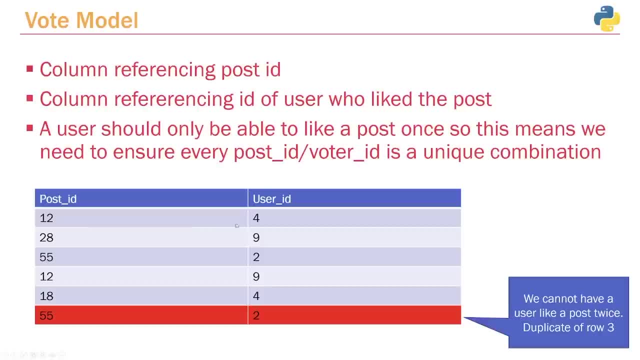 this: we have a post with an ID of 12. And this post was liked by a user ID of four. So this is what an entry would look like And that's perfectly fine. And if we go, and we here, we've got a post ID. 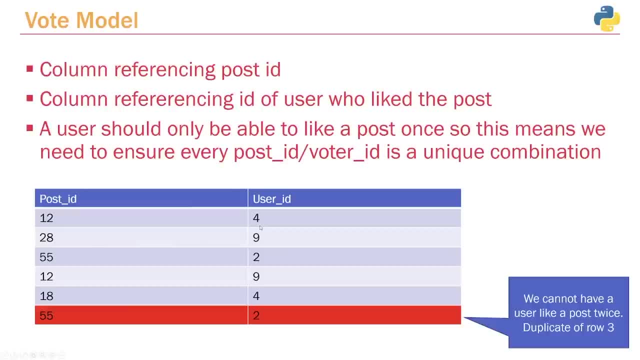 of 28.. And it looks like a user with an ID of nine like this post And if I go all the way down to here, you'll see that post ID of 12. Which you can see that there was already a row with the post. I. 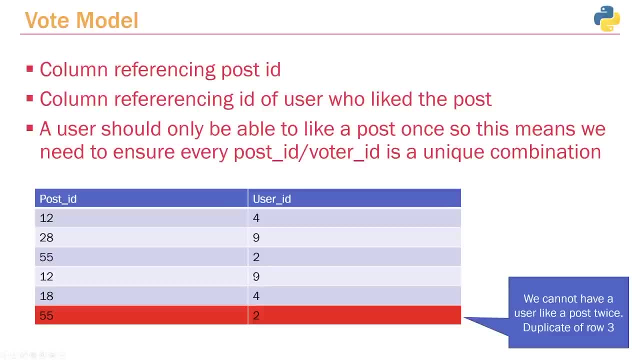 tilt is liked by a different user- nine- So it's perfectly okay to see a repeat in this column And under the user ID section, it's perfectly okay to see a repeat in this column as well, because we can see that a user of ID nine voted and liked a post with an ID of 28,, as well as a post with an ID of 12.. 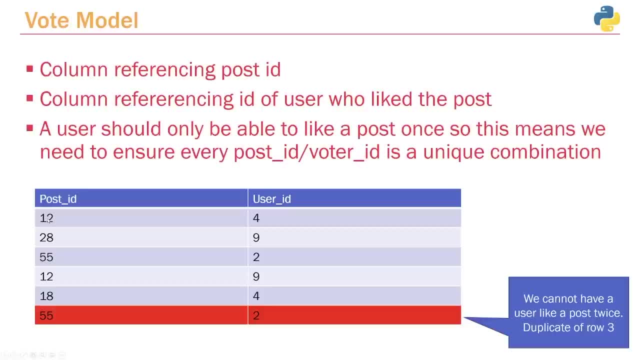 And then, obviously, one post can be liked by different users. So a post with an ID of 12 was liked by a user with an ID of four, and a post with the same post was also liked by a user with an ID of nine. Now, what we can't have is a user liking a post more than once, So you: 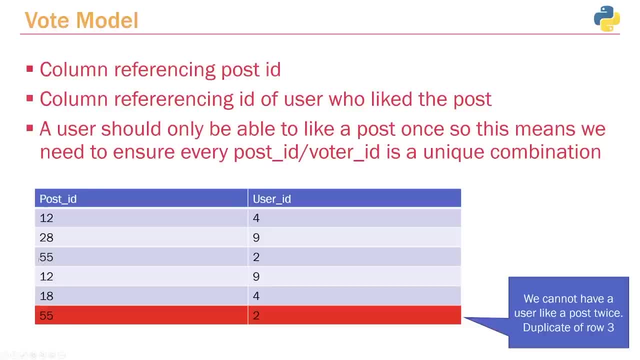 could see here user to like to a post with an ID of 55. And we can't have him do that again. Right, It's a duplicate. this isn't allowed, or this shouldn't be allowed, in our system, because we don't want users to be able to like like a post more than once, And so there's a. 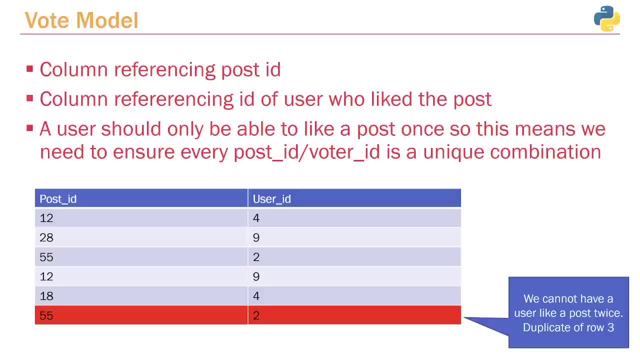 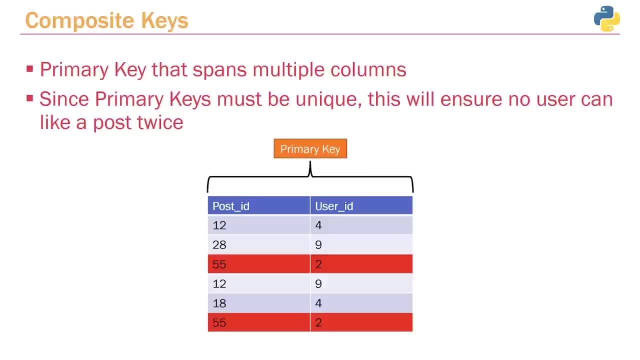 couple of different ways of setting up this requirement, But we're going to take a look at the simplest solution And we're going to learn about something called composite keys. So we've already covered what a primary key is. it's a, it's a column in your table that's going to ensure that. 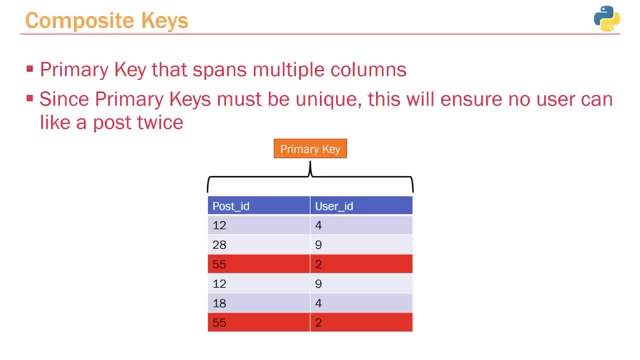 every single entry is unique, And we always used a column called ID, which had a auto incrementing integer. However, what we can also do is make use of something called composite keys, And a composite key is nothing more than a primary key that spans multiple columns, So we've only worked with one. 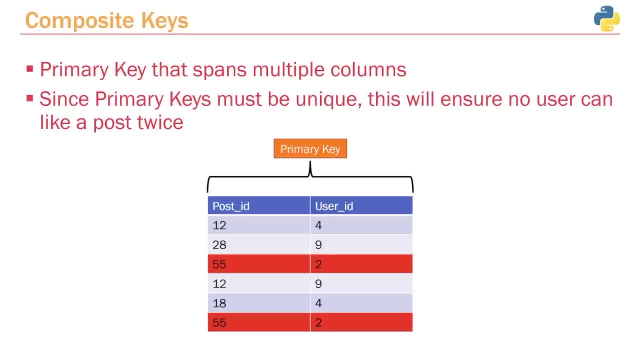 column primary keys, but we can actually have it cover more than one column. we can have two columns or three columns And since a primary key must be unique, this will ultimately ensure that no user can like a post twice if we make sure that both of these columns are part of the primary. 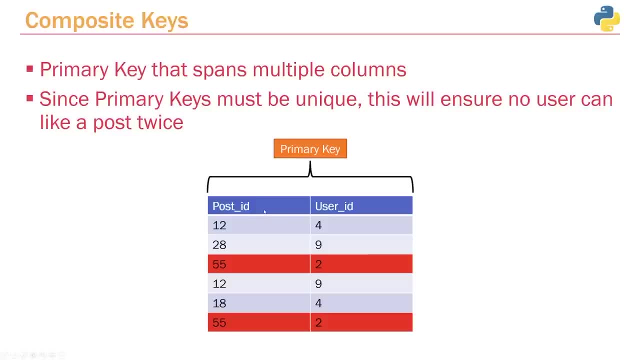 key Right, And so when you have a composite primary key, it does not care if there's duplicates in one row, it does not care if it's in one column and it does not care if there's duplicates in the other column. all it cares about is: are both of the columns? 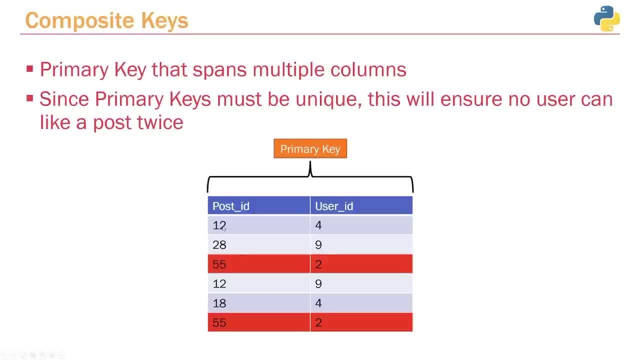 the same in two different rows. So once again, you know, for a post of ID 12, we have a user of four who likes it, as well as a user of nine that likes it, And so with a composite primary key, 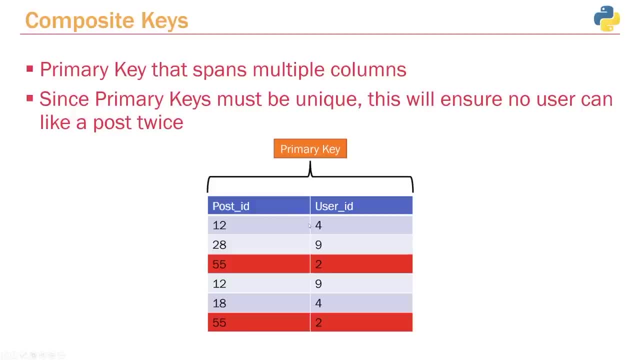 it sees that as two different entries because it needs both of them to be the same to be considered a duplicate. So we can uniquely identify this row by saying: Hey, I want the row with the post ID of 12.. And a post ID of nine. there's going to be no other rows with that combination And the same. 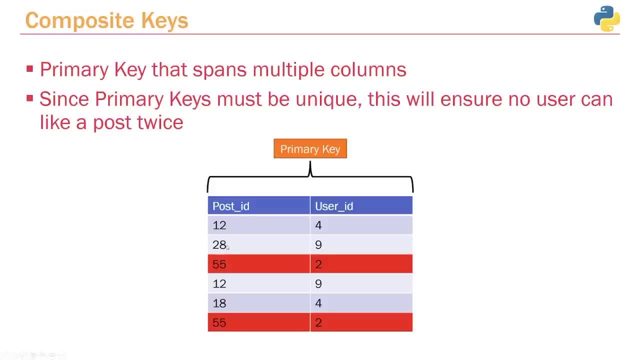 thing goes in the other direction. The user nine can like post 12, and the same thing goes in the 28. And he can also like post 12.. And so, once again, we can uniquely identify either one of these rows because we can say, hey, post a 28 with the user ID. that's a unique combination. 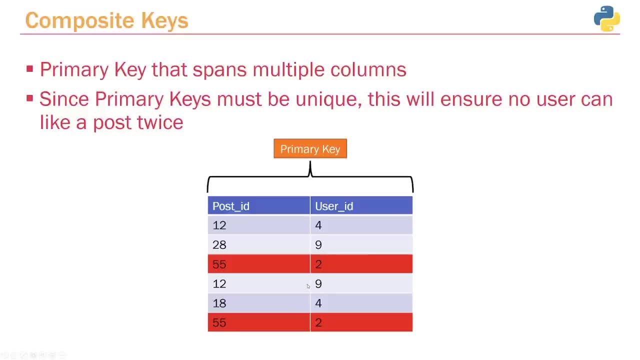 and a post ID of 12.. With a user ID of nine- once again, a unique combination. However, we can't have a user with ID of two, like 55. And then once again, the user ID of two, like 55, because 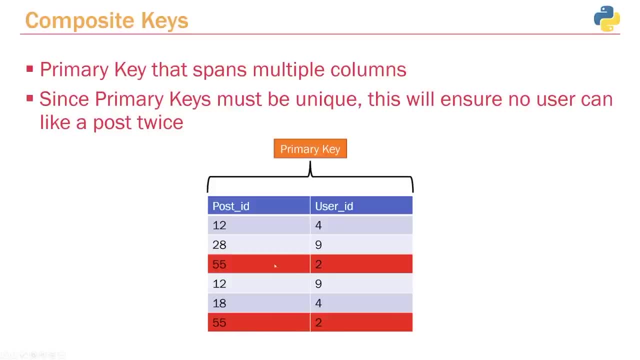 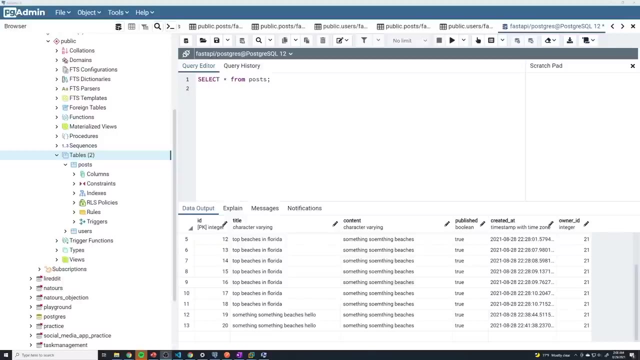 the combination of these two is now a duplicate, Because one is 55. And two and the other one's not. So that's all a composite key is? it's just a primary key that spans two columns and ensures that across both columns we have unique combinations for things. So let's figure out how. 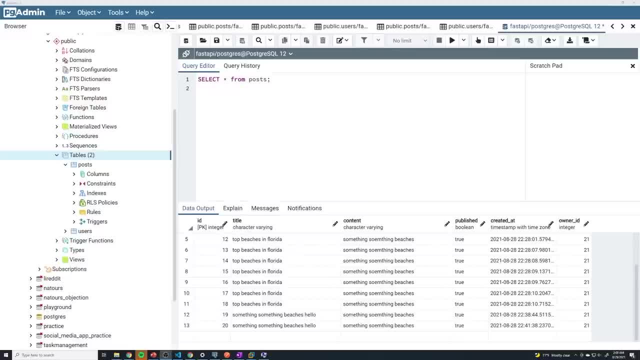 to create our new votes table And I'm going to first show you guys how to do this within PG admin, So just with regular Postgres, and then we'll take a look at how to do this with SQL alchemy And I'm just going to go under tables and I'm gonna create a new table. we'll call it votes. 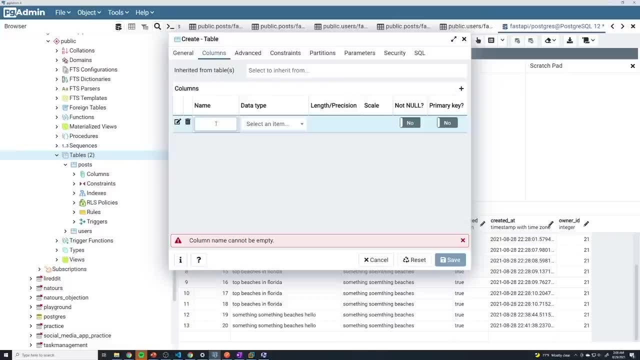 And then under columns, here I'm going to add a column And this is going to be post underscore ID. So this is going to be the column that referenced the idea of the specific post this should, and then, actually, before we do anything else, I'm going to add the other column in as: 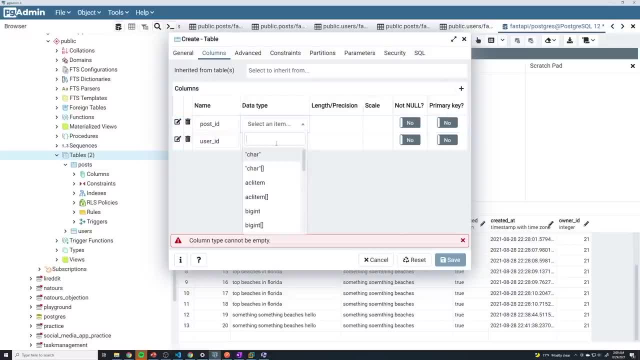 well, And then we're gonna have the user underscore ID, And so these are both going to be integers, And then we can just select primary key, primary key, And that's going to create that composite key. And then we have to set up the foreign keys as well. So these are. 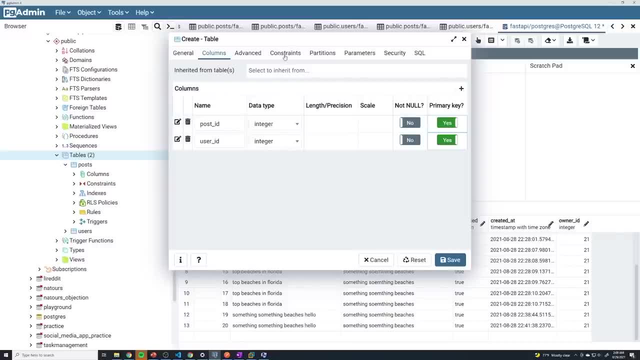 going to reference other tables. So for the post ID we can go into constraints And then we'll go into foreign key. we'll add a new foreign key And I'm going to call this: votes underscore, posts, underscore primate whoops, not primary key, foreign key. And actually sorry, I didn't mean. 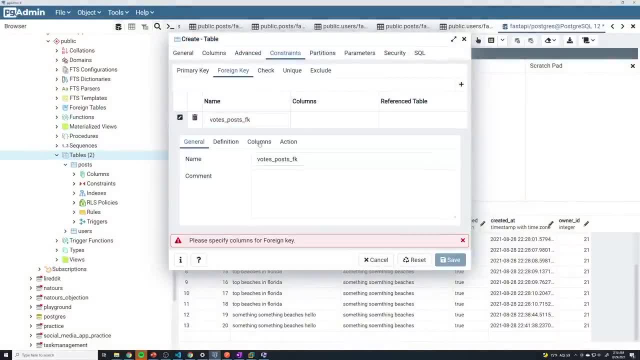 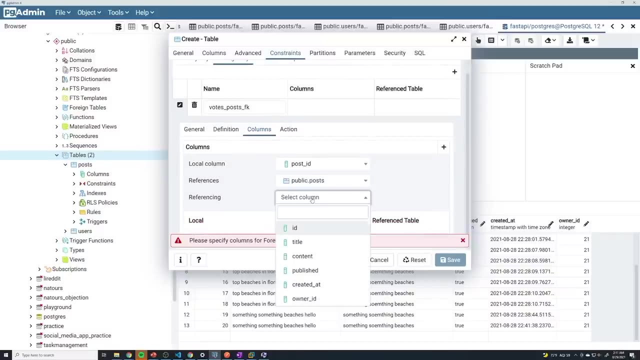 to do that, And then we're just going to go into here for the columns, We're going to select the local column, which is going to be post ID- Sorry, it's not post ID, Yeah, post ID. And then for the referencing table, it's going to be the posts table And then we're. 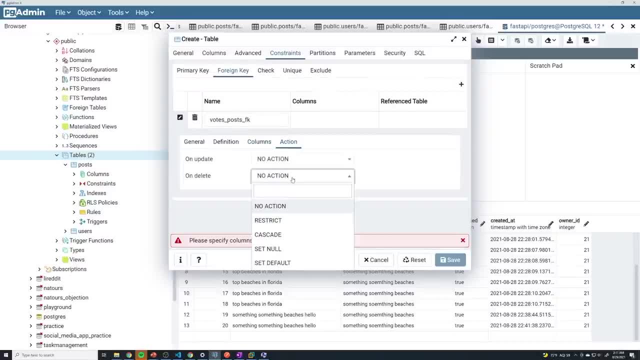 going to grab the ID of that And for action on delete, we're going to make sure it's set to cascade so that if the if the post gets deleted, we're going to delete this entry And then we'll add that in there. 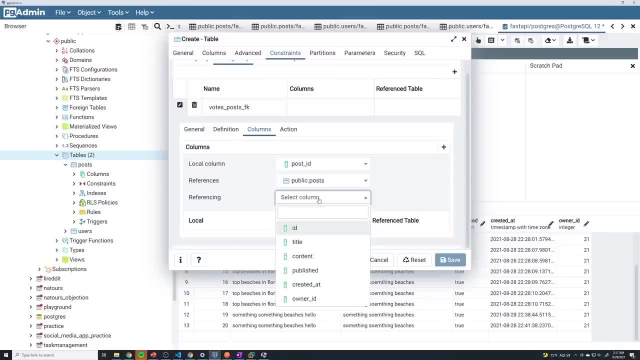 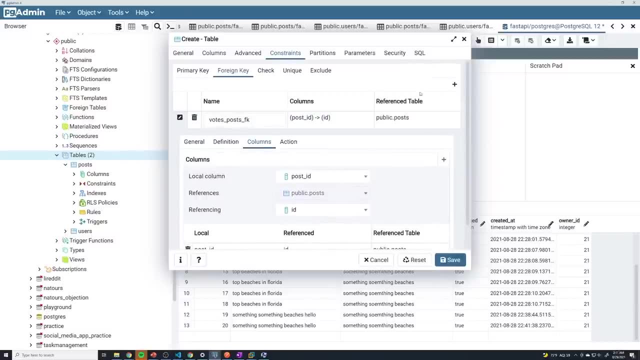 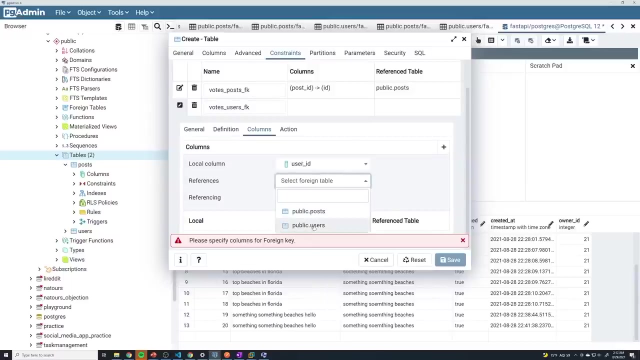 Oh, it looks like it's got deleted. Let me just redo this. We'll add that, And so we've got that in there now, And that should be it for the first foreign key. Let's add another foreign key And this is going to be called votes- underscore- users underscore- foreign key columns. this is going to be user underscore- ID of the local table. this is going to reference the users table and then it's going to reference the ID. We'll hit that. 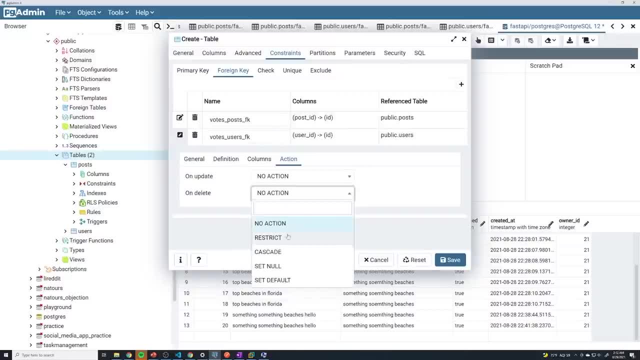 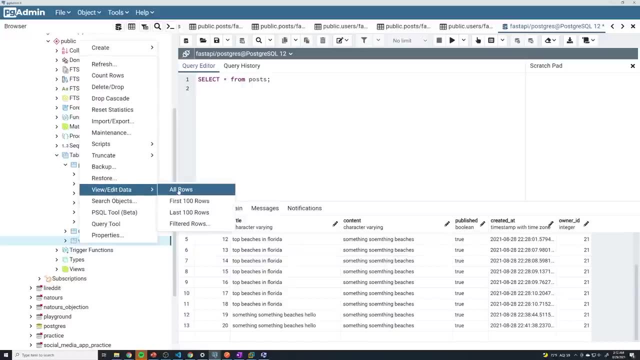 Actions. This is going to be cascade as well, And we'll save that. And then I'm going to right click on the votes table And then we can go to view edit data. we'll go to all rows. You can see, it's a very simple table, So let's create a new. 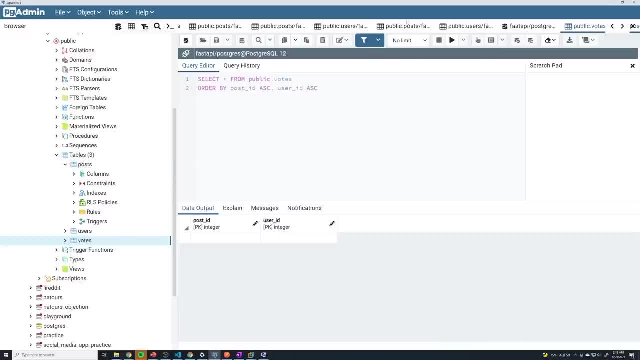 let's create a new vote first, And so I'm going to. first of all, I've got way too many of these windows. I'm going to just quickly delete those, Alright. so I got those deleted. I'm going to open up a new query. 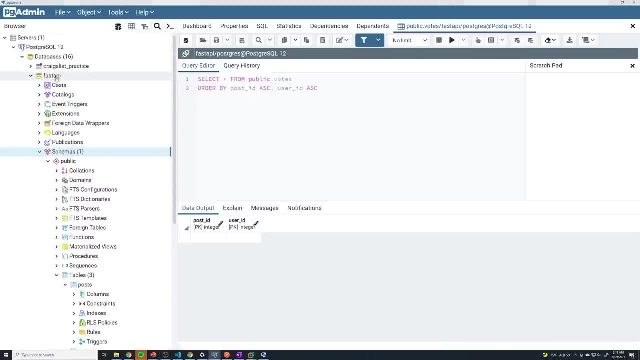 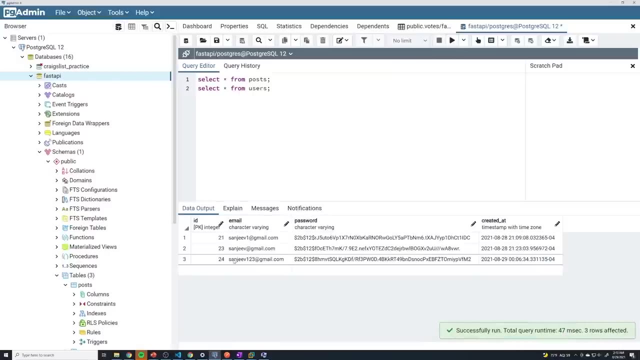 I can just go into database. we'll do query. I'm going to do select star from posts and then select star from users, just so I can get a list of post IDs and user IDs. So I got user ID of 2123, 24.. And 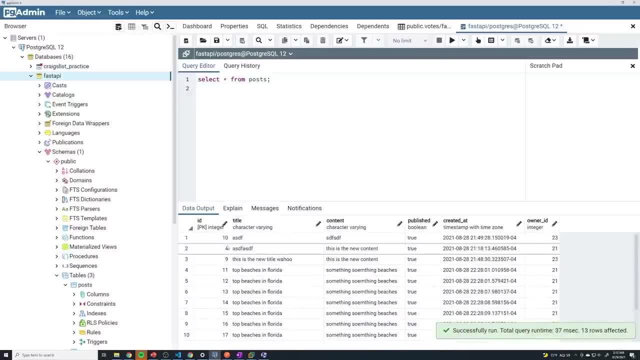 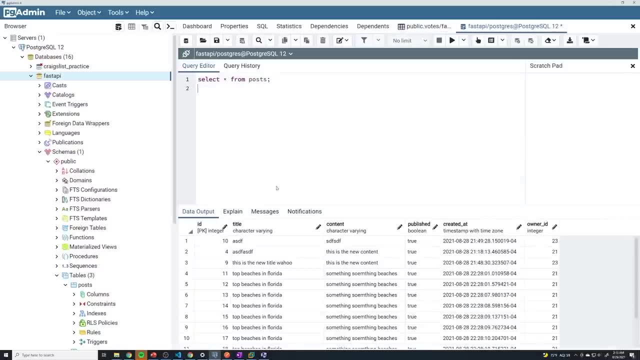 for the post, we get 1049.. So let's try those out. And I already forgot them. So let's, let's get that post ID again. So we'll just grab a post ID of 10.. There's going to be 10 and then the user ID. Well, I'm going to open up a new window so I can just switch between them. 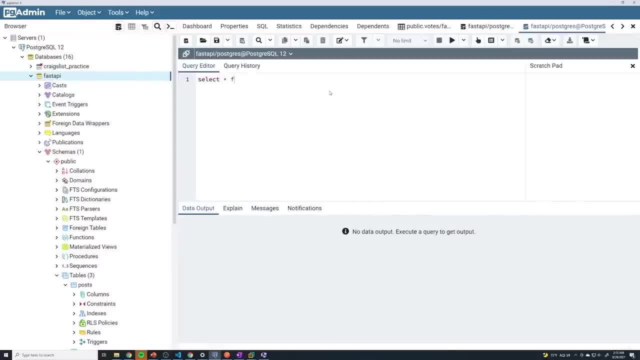 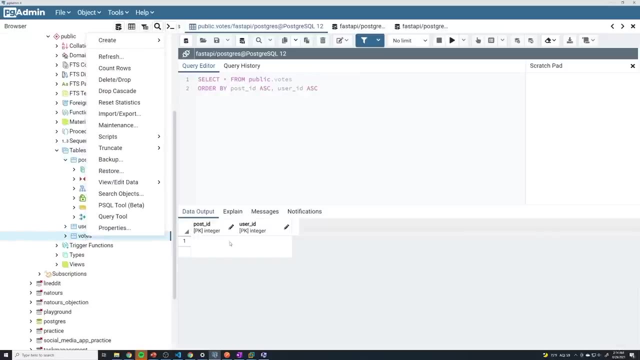 So now we have the both of these windows for querying and I can do select star from users 21.. Okay, so we'll do. And it looks like we hit a bug in PG admin because I can't write anything here, So I'm just going to do view, edit data, all rows again. 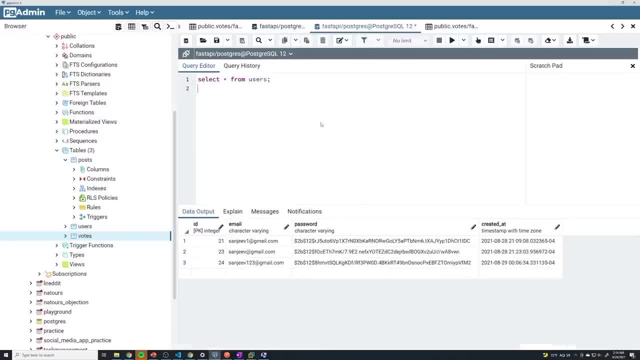 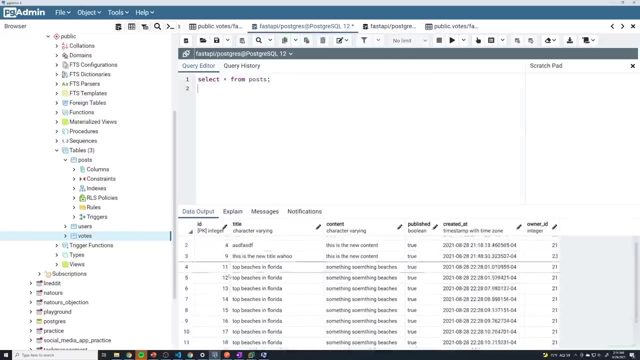 And that looks a little bit better. So let's get a post 10 and a user of 21.. 10- 21. And let's see if we're successfully able to get that and looks like that worked. And then if I grab a post ID that doesn't exist, So let's say like 99. 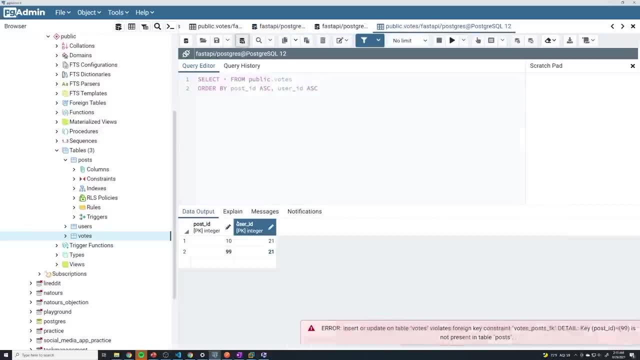 21.. And then a valid user. Let's see what happens. It's going to throw an error. That's good. And if we grab a valid post number but a ID of a user that doesn't exist, we should also get. 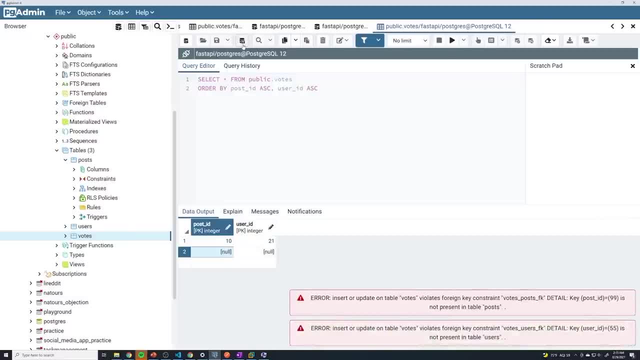 an error And then, if any of these are blank and save, it should throw an error as well. Okay, so our table looks set. That's pretty much all we have to do. There's nothing else for these tables. You'll see that once you can create one table, you can really create them all, So I'm just going to drop this table for now. 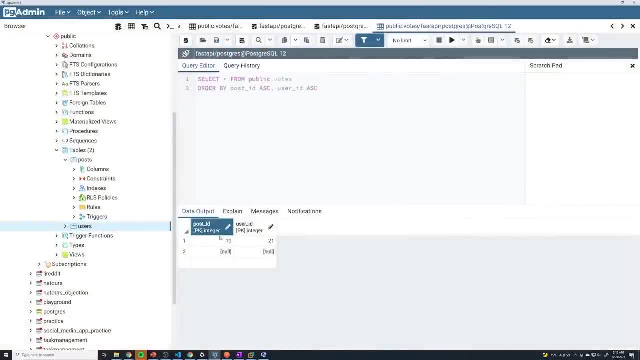 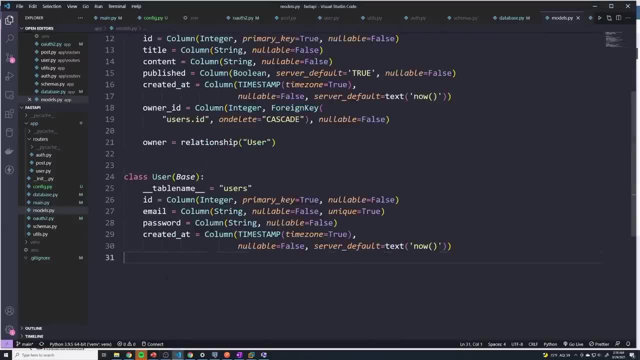 And in the next video we'll take a look at defining our model and SQL alchemy so that SQL alchemy actually generates the table for us. In our modelspy file let's create our model for our votes table And we'll call it votes or just vote. It's going to extend base. 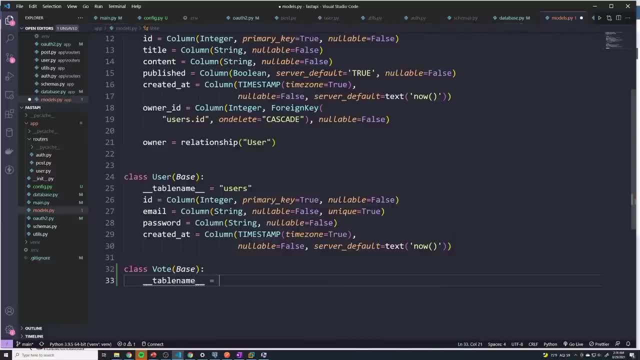 And then for our table name- I think it just makes sense to call it votes. Then let's set up our two columns. So we're going to have a user ID And then we're going to have a post underscore ID. So for the user underscore ID, it's going to be a column. 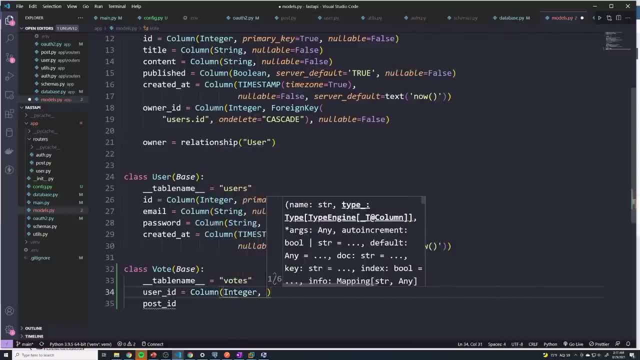 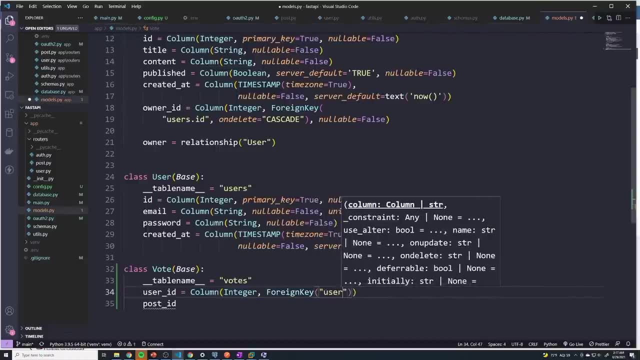 And it's going to be of type integer. We're going to set up the foreign key And this will be users, So it's going to reference the users table and grab the ID field And then the second Property is going to be the on delete, which is going to be set to cascade. 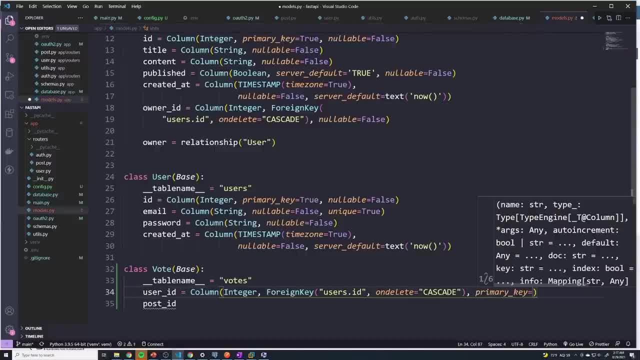 Right, then we'll set the primary key to be true, And that's pretty much it. And then I'm just going to copy this, Paste it here. We're just going to change this to be, instead of users ID, we're going to be: it's going to be postsid. 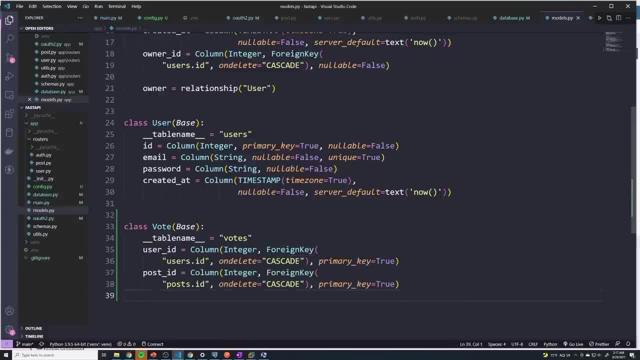 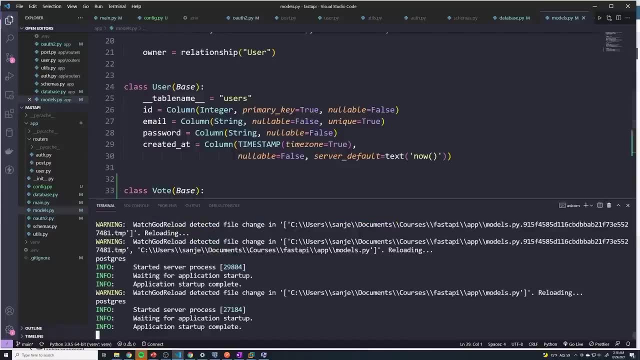 And I don't know why, I got auto formatted to a different line. Okay, Okay, It looks like That's what it prefers, And so save this And, assuming there's no errors, Our application should restart And then, if we go to PG, admin. 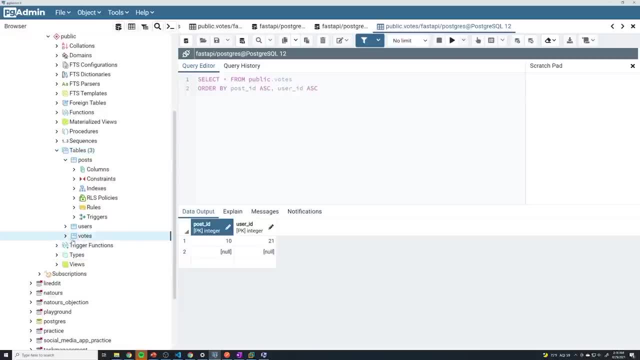 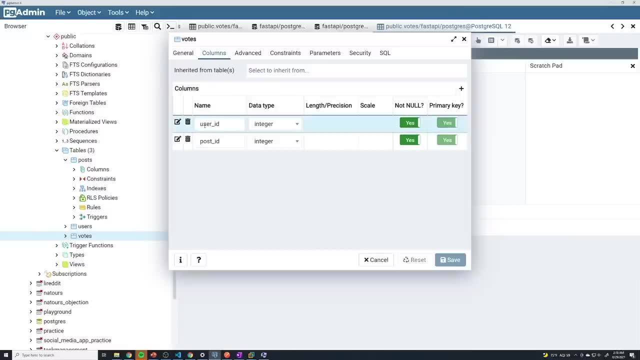 And then refresh. We should see a votes table And I'm just going to go and take a look at the properties And you can see that we get the user ID and the post ID. We've got the primary key set, So it's a composite key And since it's a primary key, not null is going to be set to. yes. 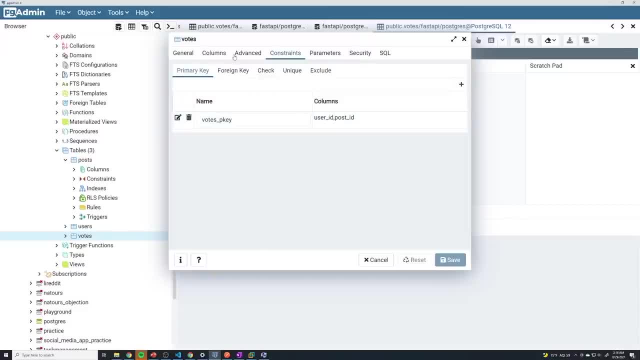 We go to constraints. We've got you know once again, both the primary keys. we should have two foreign keys And then if we just take a look at one of them real quick, we should see cascade on delete. And so if we go and view and edit data, 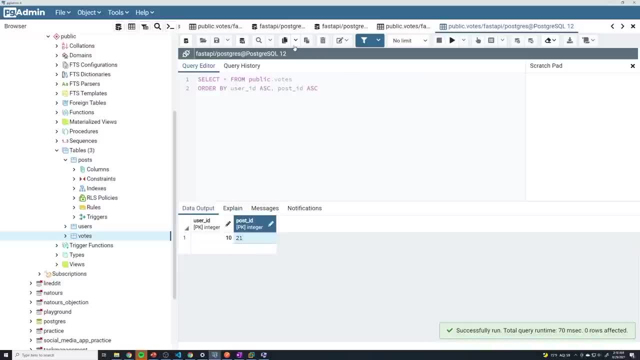 Let's test this out: 10, 21 again. So it should be 21 and 10, because the user ID is the first column. now 21,, 10.. Let's try saving that. Good, Let's try doing 21 and 9.. 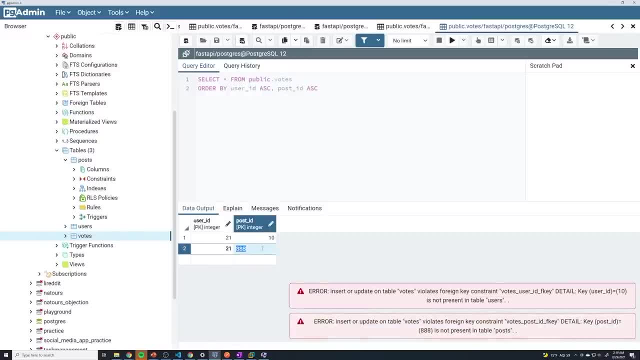 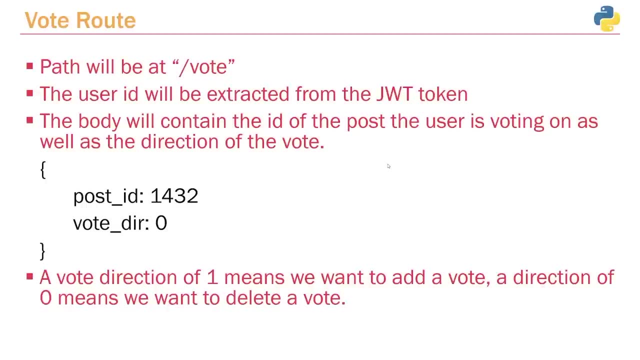 Or 21 and 88. Should error out, Perfect. And then let's try 10 and some random number: Error Perfect. Now there's going to be a couple things that we need to take into consideration when setting up the vote route. 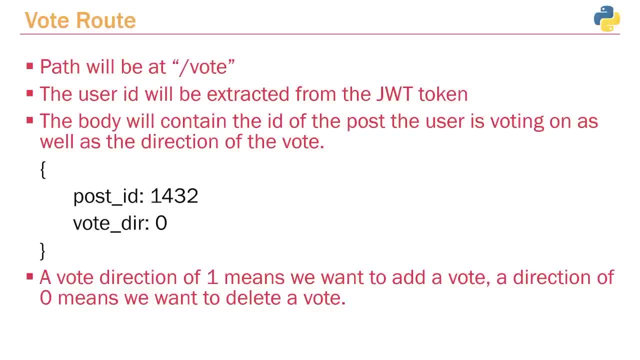 So, first of all, what is the path we're going to use? And I think it makes sense just to set up a new path called slash vote, Just like we have for slash users when it comes to handling anything with users, And we have slash post for handling anything with post. 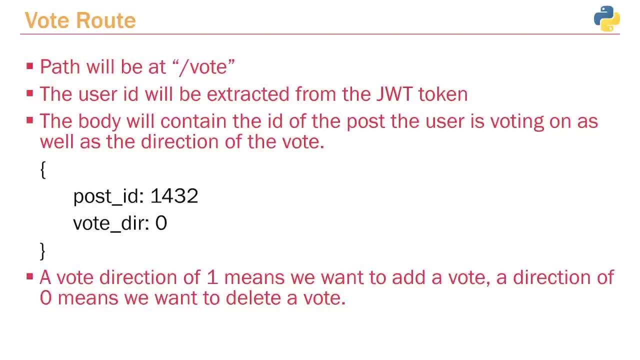 We're going to have the slash vote for handling voting Now. the user ID, the user who's trying to vote on or like a post. the ID of that user is going to be extracted from the JWT token, So we don't actually have to extract that from the body. 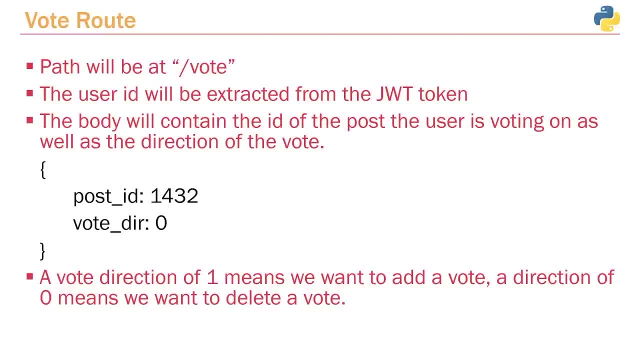 We don't need to include it in the body. However, the body itself is going to contain two pieces of information: The ID of the post we're trying to like, as well as the direction of the vote. And what I mean by direction is: do they want to vote on the post? 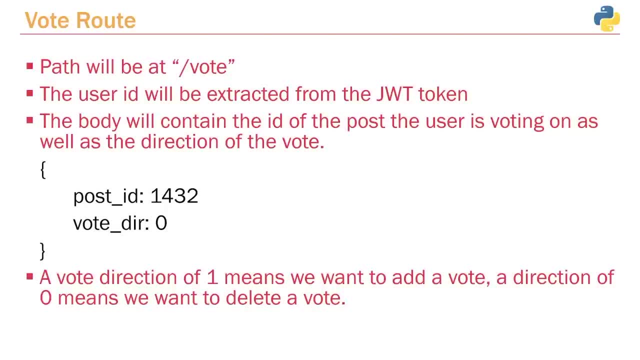 Or do they want to remove a post? Because, like any application, you know maybe you accidentally clicked on a post to like it, but you realize you don't want to like it, So you click on it again to remove that. So vote direction of one means that we're going to like the post. 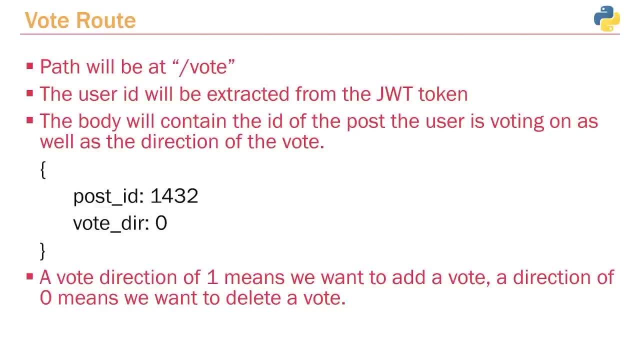 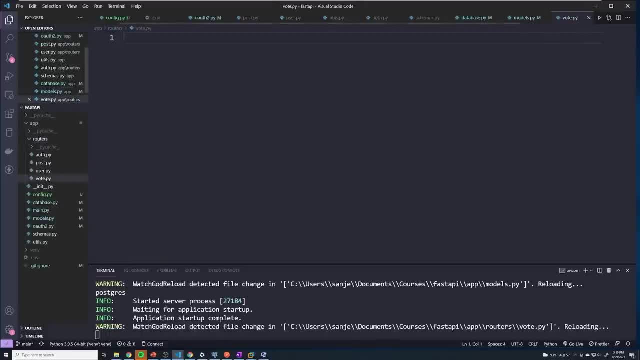 And then a vote direction of zero means we're going to remove our like of the post. Now in our routers folder we're going to create a new file which is just going to be votepy. So this is going to handle all the routing for our voting URLs. 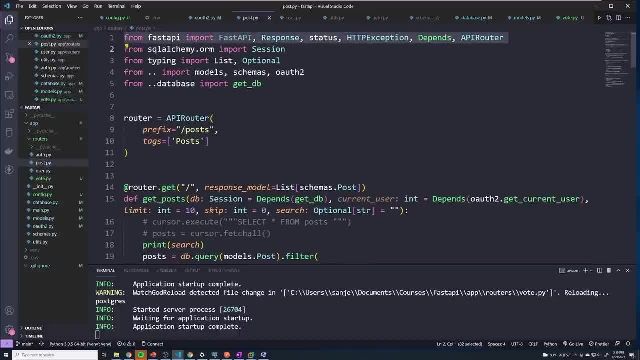 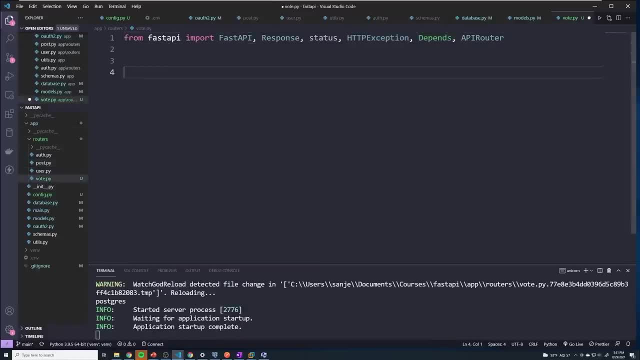 And what I want to do is I'm just going to copy the import statement from one of the other routers And we'll set up our route. So let's set up the decorator first, And this is going to be a post, And I actually have to import router. 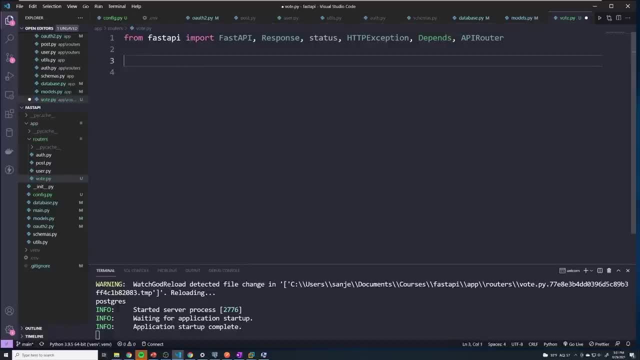 And we got it. Let's create our router instance, So we'll say router equals API router And we'll set up the prefix to be slash vote and the tags: We're going to give it its own section which is going to just say vote. 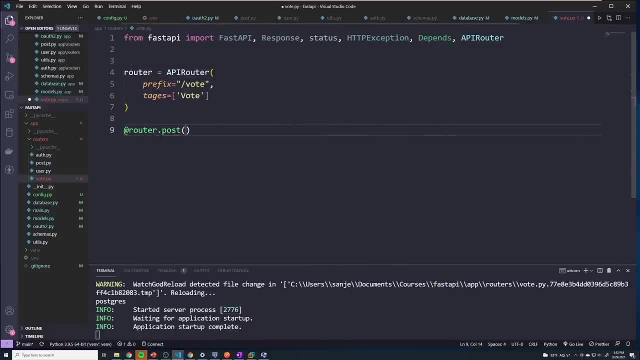 And so now we can do at router dot post. This is going to be a post operation because we have to send some information To the server and the the URL is just going to be slash. So it's just going to be slash. vote then. 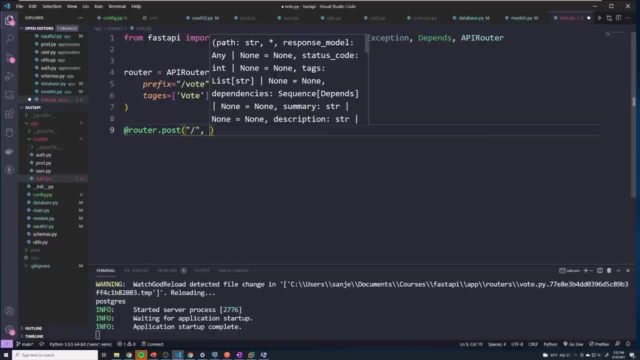 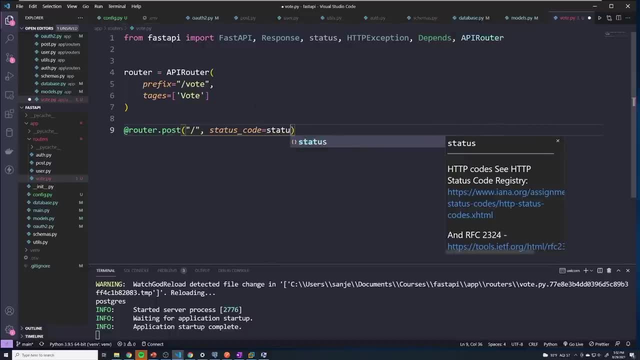 And since we're going to create a vote by default, we're going to send a different status code. We're going to send a 201 instead of the default 200.. And then we'll define our function, which I'll just call a vote. 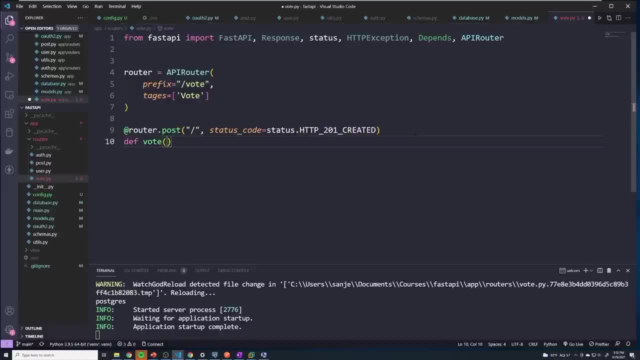 Now there's going to be a couple of things that we have to pass in. So, since we expect the user to provide some data in the body, it usually means we want to define a schema just so that we can ensure they send us the exact information. 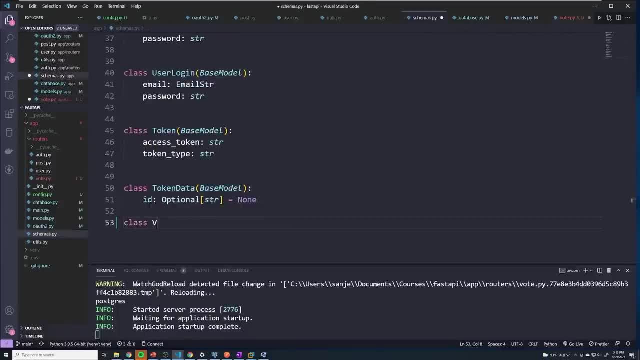 So let's set up our schema for voting. We'll create a class called vote, And so the first field should be a post ID, which is going to be of type int, And then we're going to have a direction, Which is going to be an integer as well. 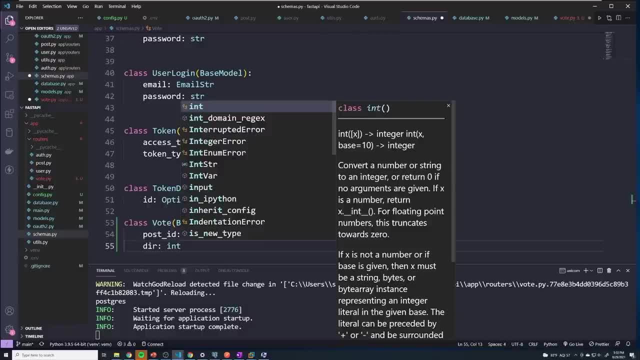 So it's either zero or one. However, I would like to be able to validate it to ensure that it's only zero or one. I couldn't exactly figure out if there was a way to do that in Pydantic, But one thing we can do is we can use a continent. 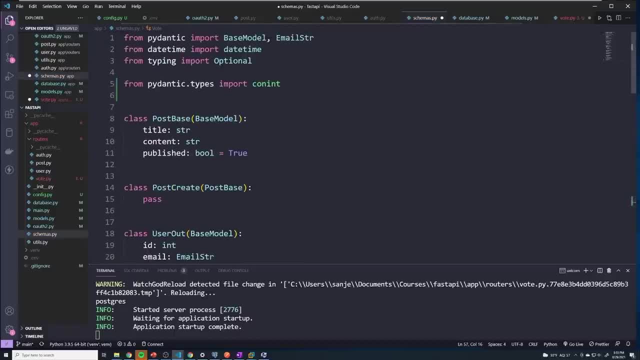 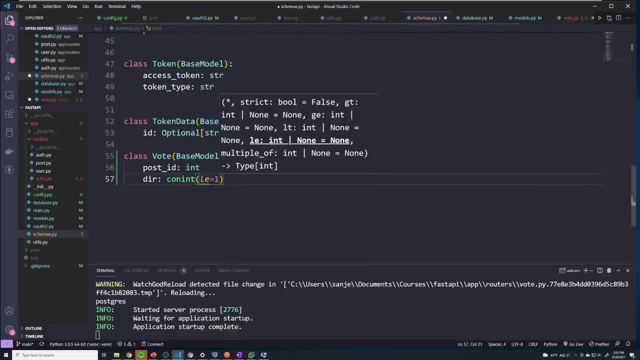 So we will import that from Pydantic automatically. So if you want to see the import, that's what it's going to look like, And we can say less Then, Or equal to one, So anything less than one is going to be allowed. 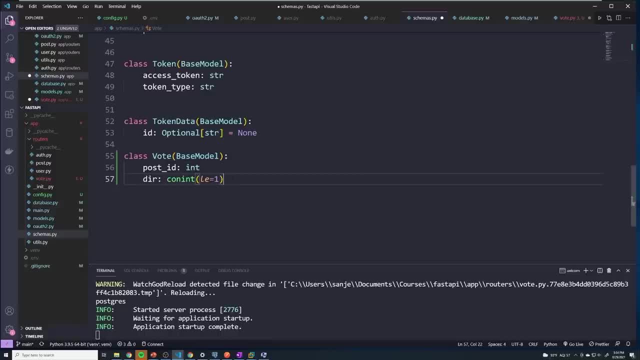 The only problem with this is that allows for negative numbers. But that's OK. You know, if you guys figure out how to just specify zero on one, then you know, go ahead and replace that and definitely leave it. Leave that piece of information in the comments so that anyone else who wants to set up that specific restriction then we all know how to do that. moving forward, 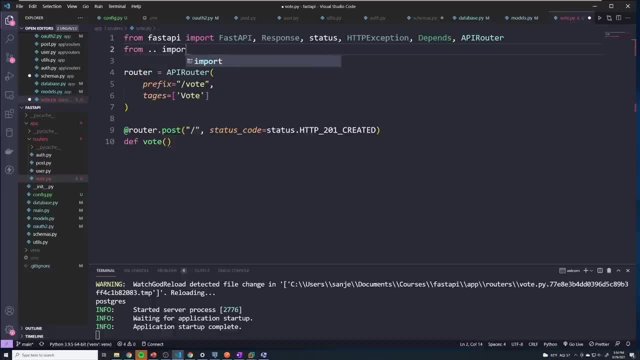 And let's import our schema now. so we'll go up A directory And let's also import database Models, and we're going to have to require the user to be logged in before they can vote on something. So let's import a lot too. 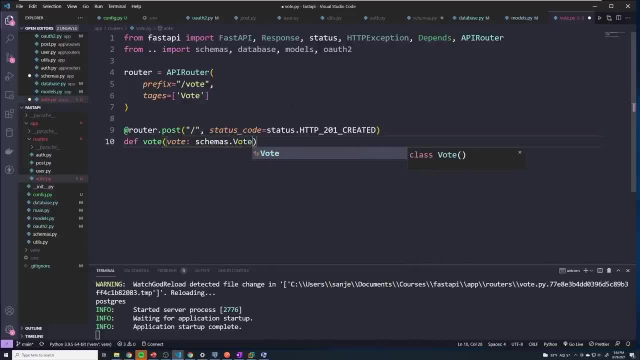 And so here we're going to set up the schema And we're also going to set up the database so that we can make queries. So let's just say we want to do a question on this ind5 Android, So we'll say: And then, lastly, we'll get the current user. 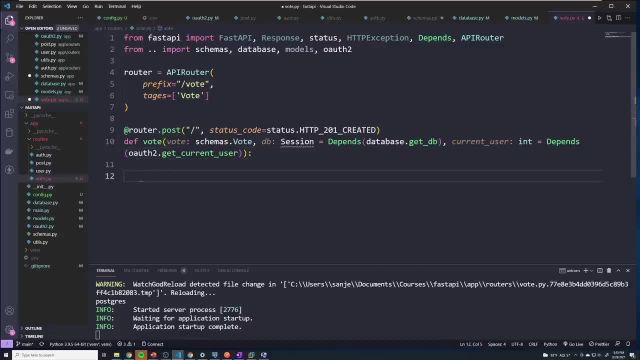 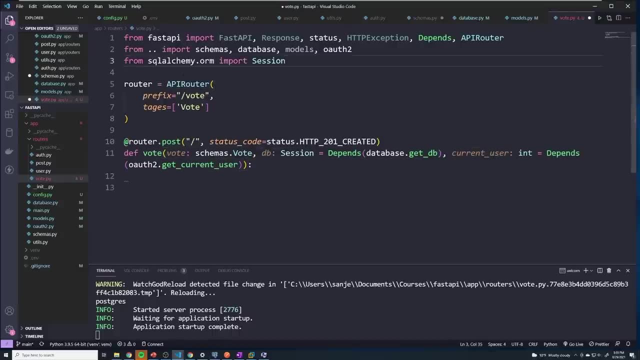 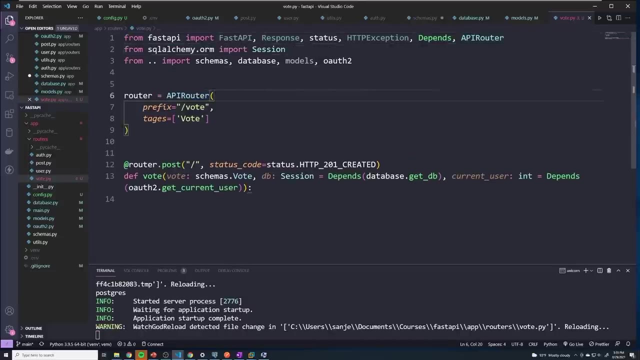 And then, lastly, we'll get the current user. Okay, all those dependencies looks like we have to import session as well, And I'm actually going to move this right below the first import. not that it matters, but- and so we're going to set. 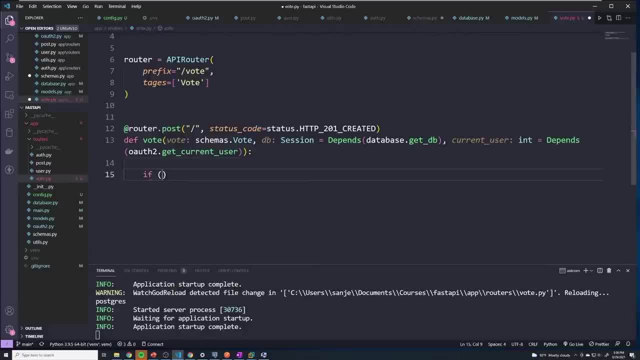 up logic for when the vote direction is one. So if I, if vote dot dir, so we're pulling the direction from the vote schema equals equals one, then we're going to perform some logic. Else, if it's zero, then we're going to perform some other logic. So if we want to create a vote, 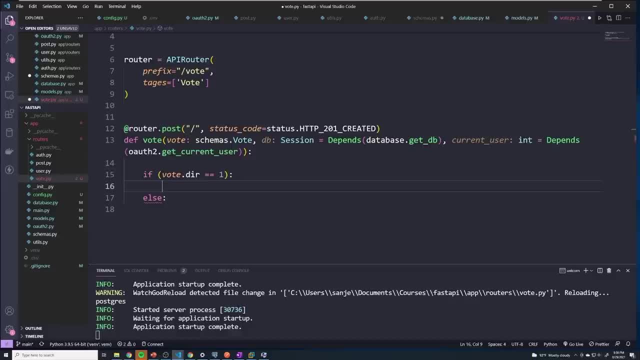 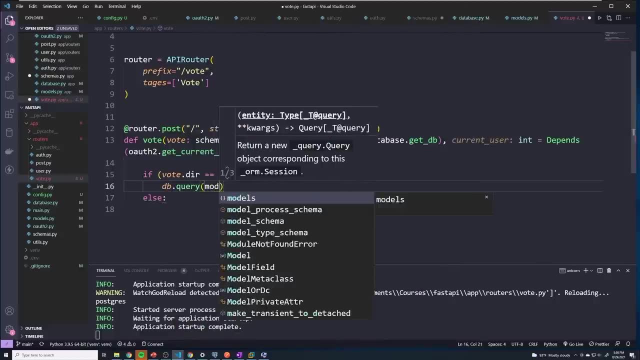 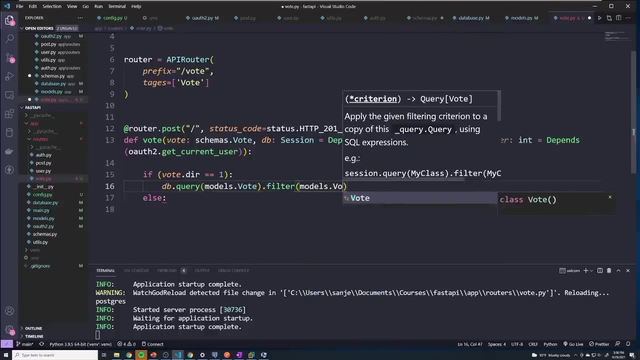 the first thing we're going to do is query to see, you know, does the vote already exist? And so what I'm gonna do is I'm gonna say DB, dot query, And we'll grab models dot vote. And I'm going to filter based off of models dot vote, dot post. underscore ID. 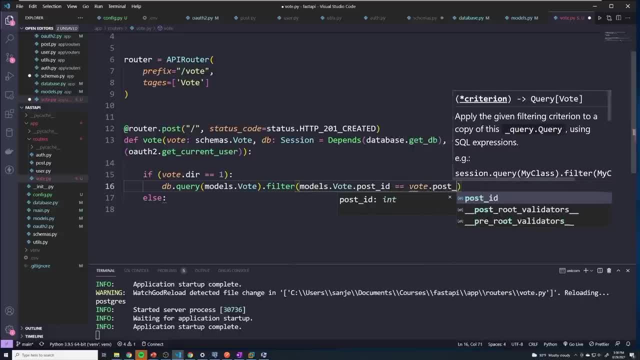 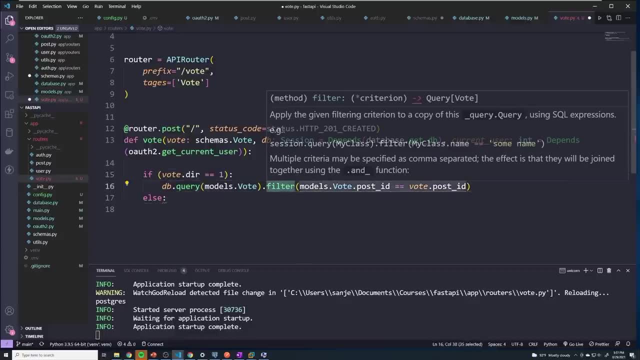 And we're going to say it equals equals vote dot. post underscore ID. So we're going to see if there's already a vote for this specific post ID. However, this isn't enough because, remember, multiple people can vote on the same post, So we actually have to do a second check. 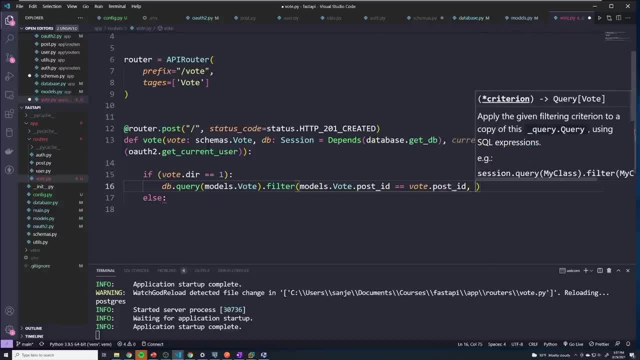 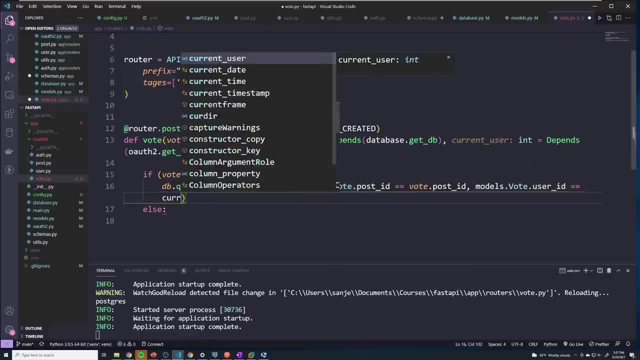 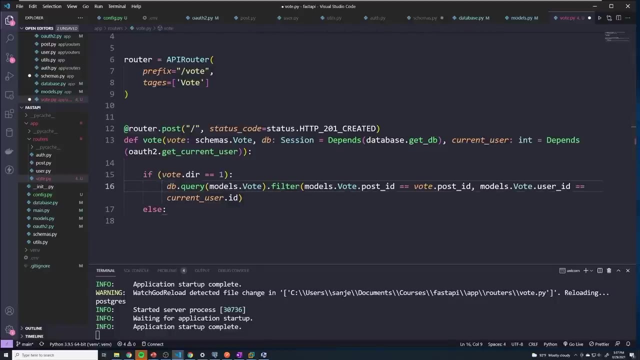 And we can add in a second condition by just doing a comma and then providing the second condition. So we have to say: models dot vote dot. user ID equals equals current user dot ID. And I'm going to save this and we're going to call this vote underscore query. So this isn't. 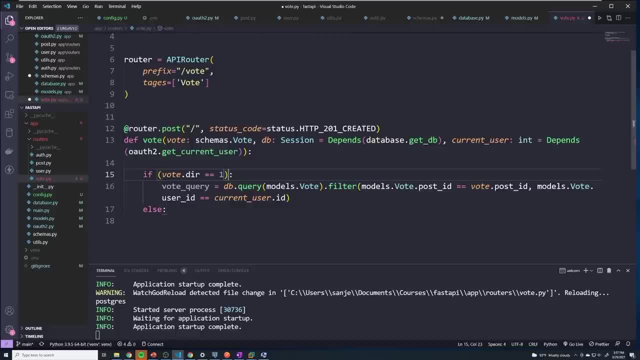 going to actually query the database yet. This is just building out the query And it's going to check to see if this specific user ultimately has voted for this specific post already or like this post. And I'm actually going to move this above the if statement And you guys will see. 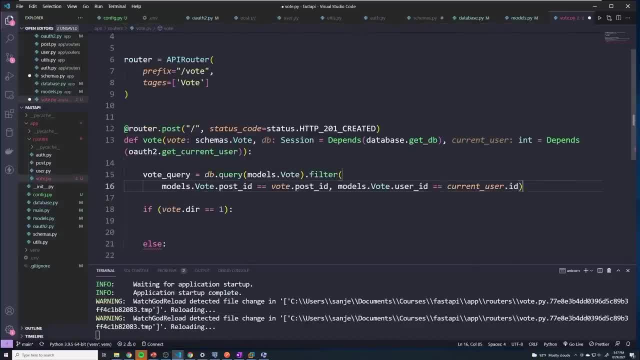 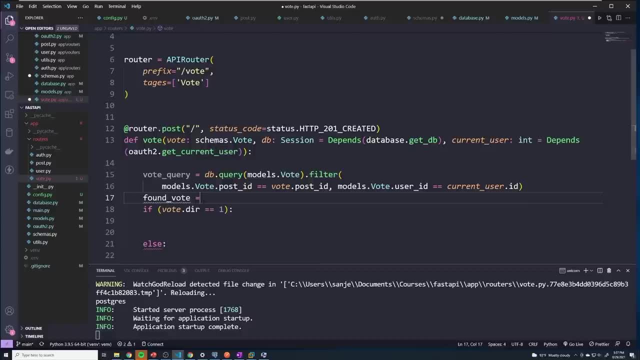 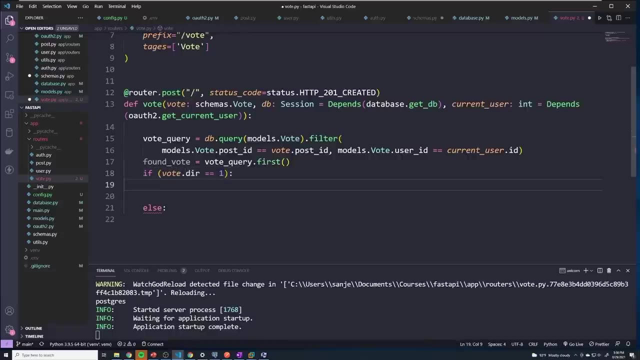 why we're going to do that in a bit And we're going to then perform the query, And we're going to perform the query and just save that result under found vote. equals vote underscore: query dot first: Alright, and so if the user wants to like a post, but we already found a post, 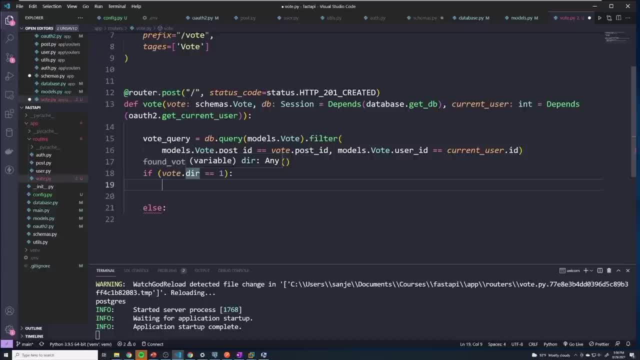 that means he's already liked this specific post, so he can't like it again. So we're going to say: is if we already found a vote, then we're going to raise an HTTP exception. Now the status code: we're going to use a new status code I'm going to use. 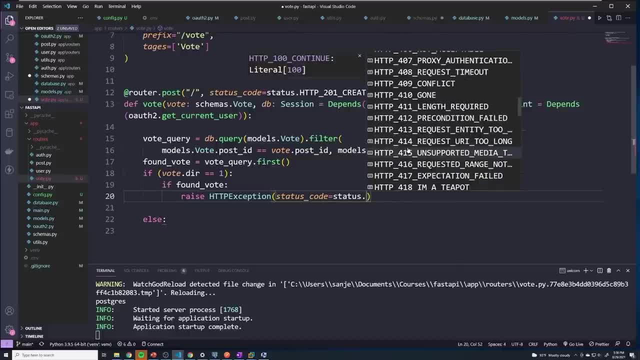 status dot and then this status code. we're going to use a new status code. I'm going to use status dot and then this is going to be a 409.. A conflict, and there's other status codes you could potentially use. 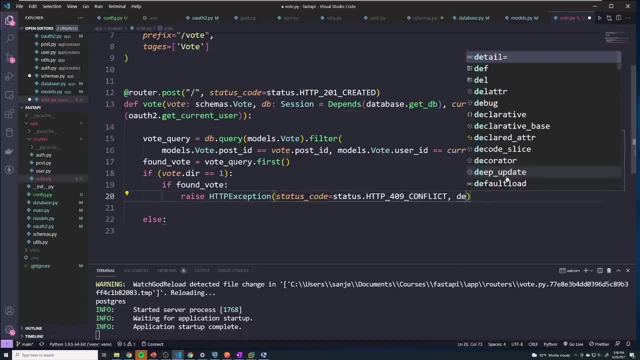 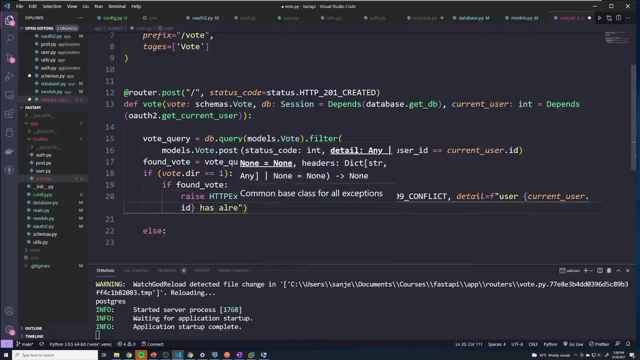 I just decided that this is probably going to be the best fit And then, for detail, we're going to just pass an F string and say user, And then we pass in the user which is get current underscore. user dot ID has already voted on post with an ID of. 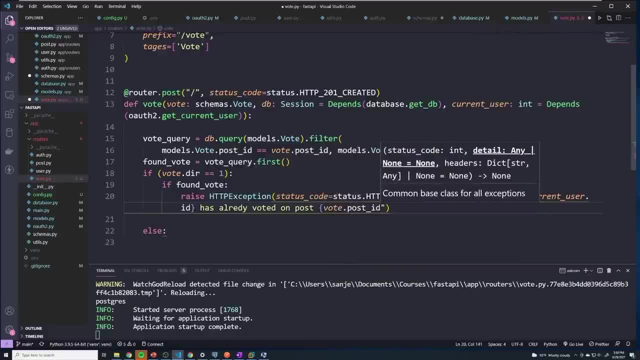 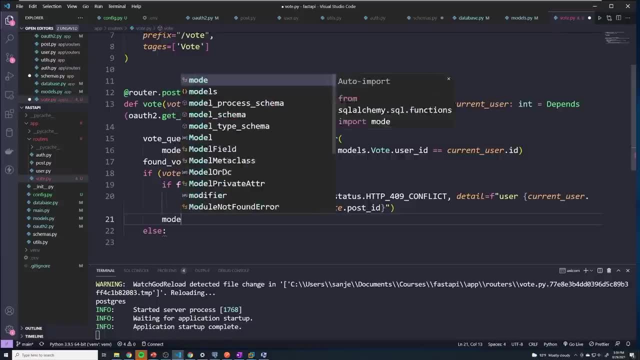 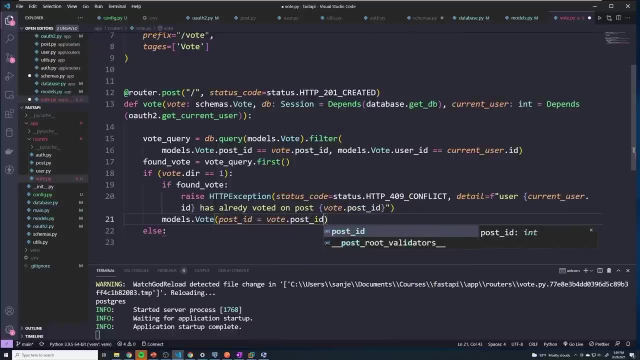 vote dot post underscore ID. Alright, but if we didn't find a vote, then what we're gonna do is we're going to create a brand new vote. So I'll say models dot vote, And so the post ID field is gonna be set to a vote dot post underscore ID. 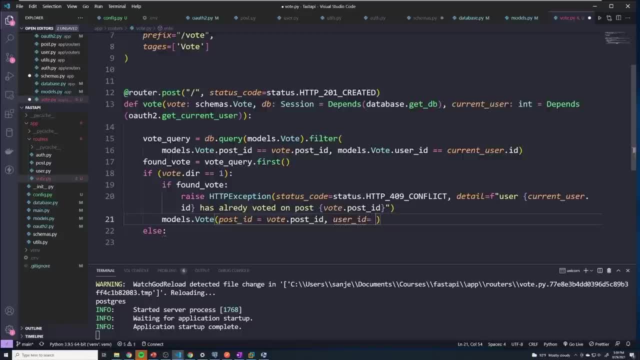 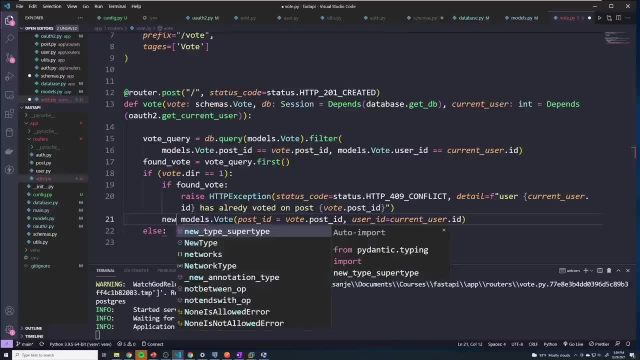 and then we can grab the user ID field from current user dot ID. So this will set the two properties And we'll save this as new underscore vote And, as usual, to actually perform these changes or to add this to our database, we have to. 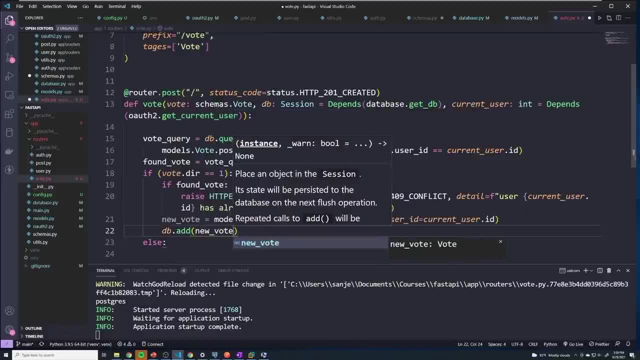 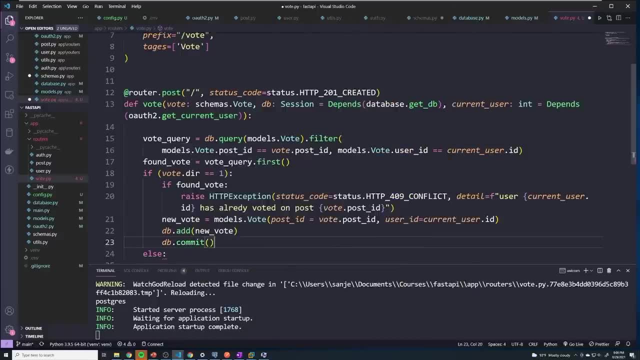 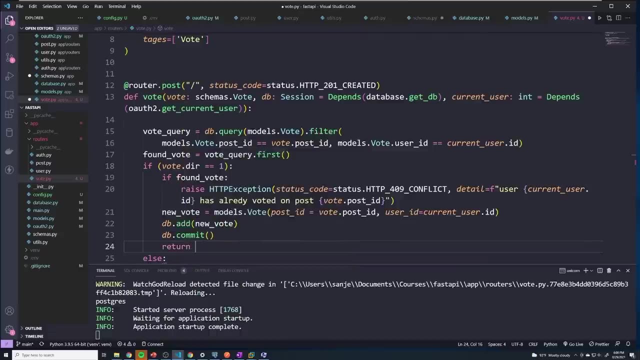 do DB dot add new underscore vote and then a DB dot commit, And we don't actually need to send the created vote back to the user because it doesn't really provide any useful information. So we're just going to send a message that says successfully added vote. 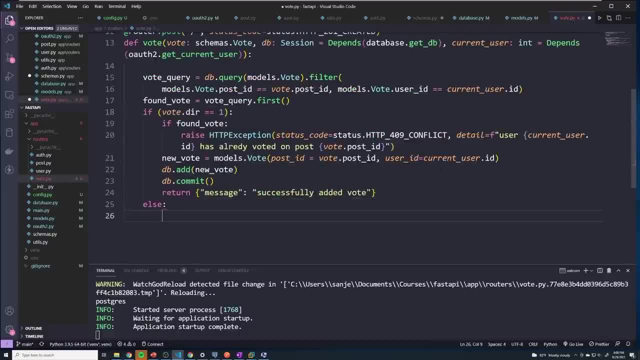 Now, if the user provided a direction of zero, that means they want to delete a pre existing vote. So first of all we'll say: if not found vote right, we can't delete a vote that doesn't exist. So we'll raise an HTTP exception. 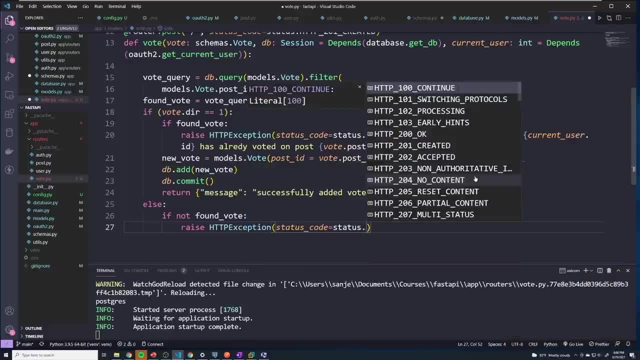 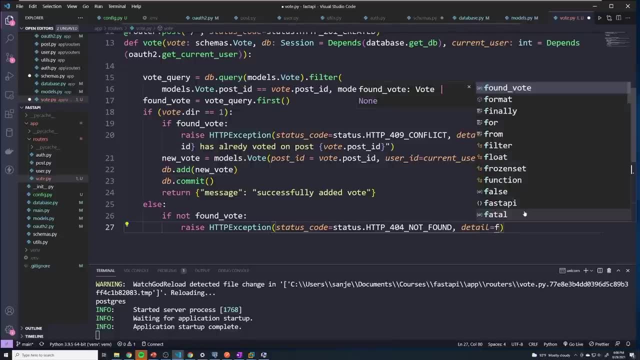 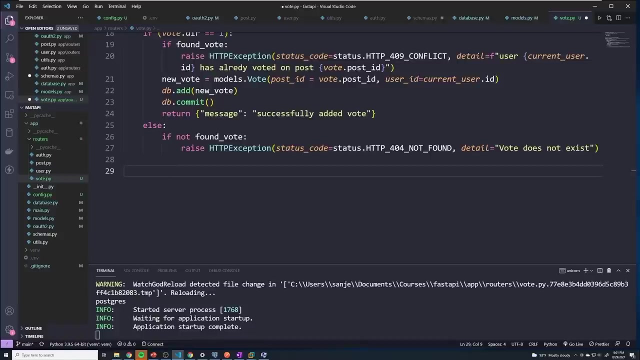 status code. I think we could just send a 404.. And for the detail, just say a vote does not exist. But if we did find a vote then we have to delete it. So I'll say vote underscore query. Remember this is a query, all the way at the top. 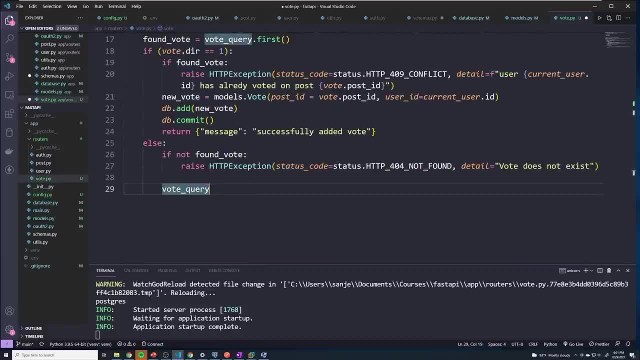 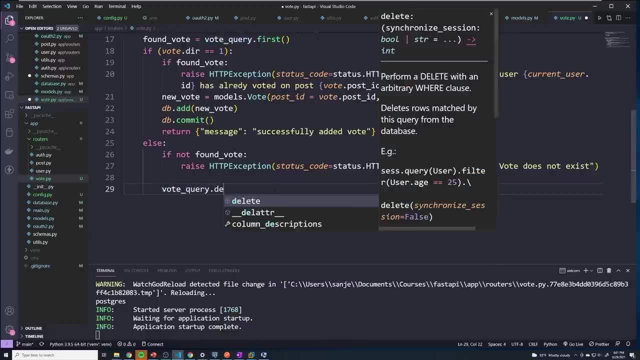 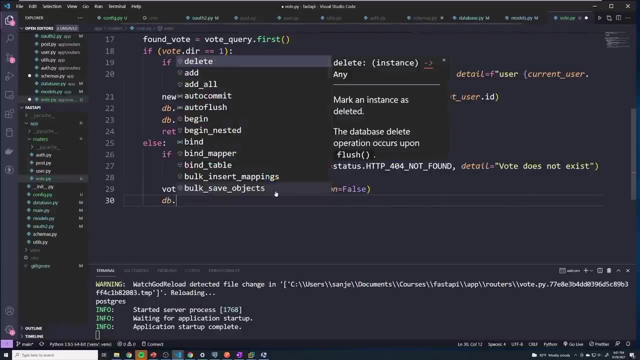 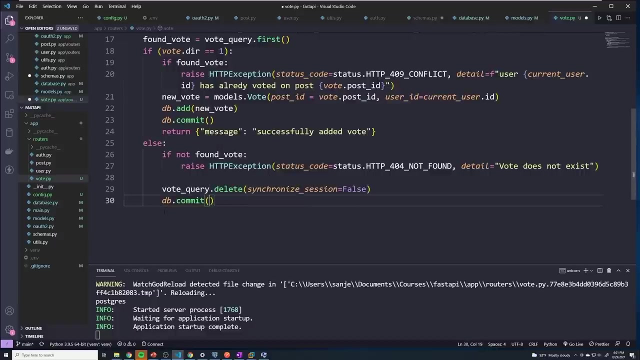 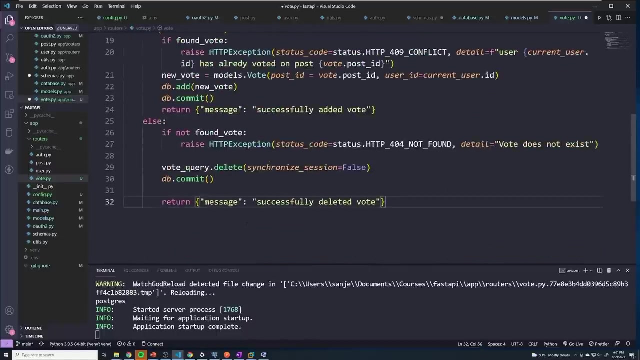 I'll say dot delete And then we can just do our synchronous synchronized session false And we'll do a DB dot commit And we'll just return a similar message: Successfully deleted vote. Okay, and this should kind of sum up all of the logic in our path operation function. 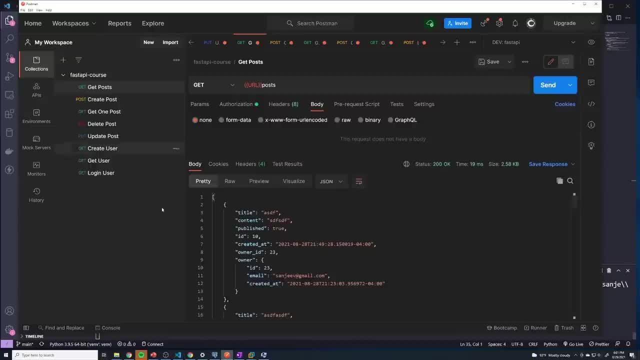 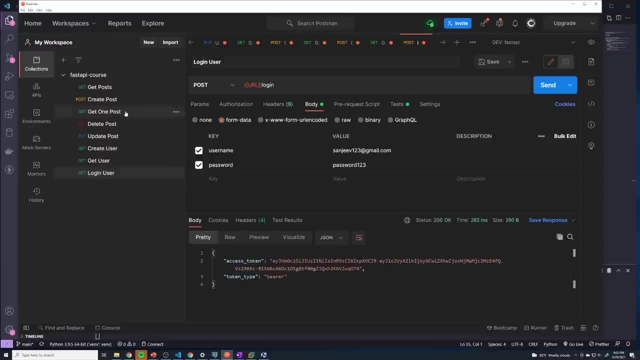 And at this point we can just go ahead and test this out. So we'll go back to postman. First of all, let's log in. Alright, so we've logged in And what I'm going to do is create a brand new request. we'll call this vote. 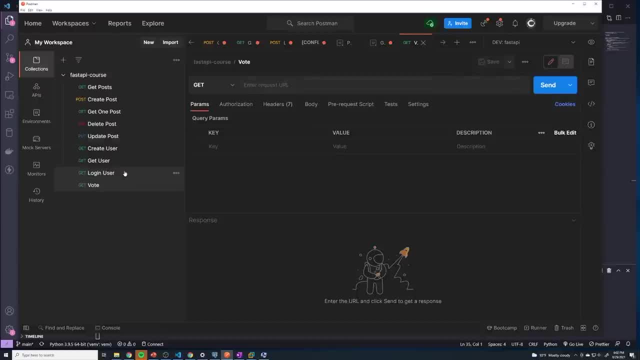 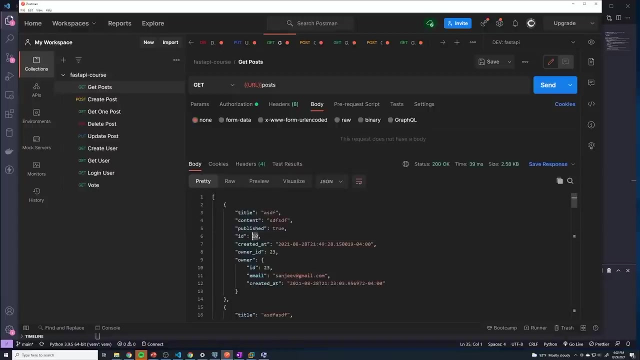 Okay, And this is going to be a vote, And in the body we have to pass in the specific data. So let's actually grab a post or an ID of a post. So in this case there's an ID of 10.. 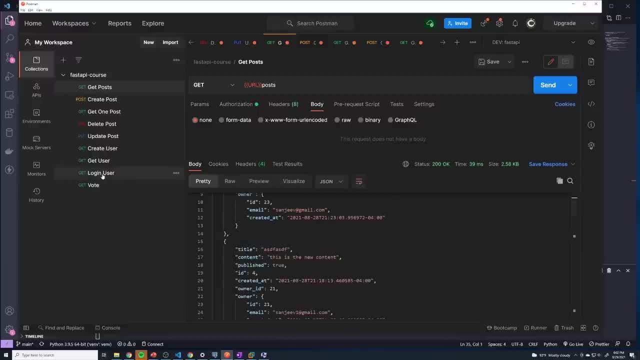 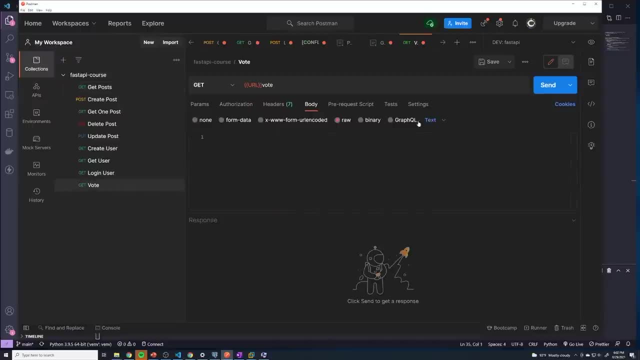 Actually, first let me double check who I'm logged in as. Okay, that's fine. So I'm going to grab a post with an ID of 10. here we'll say post underscore ID 10.. And then we'll say: der, actually, is that what we called it. 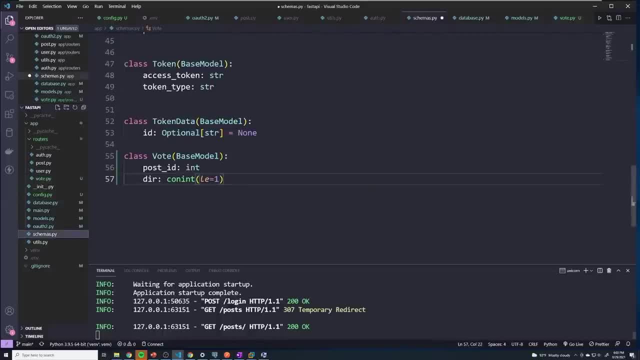 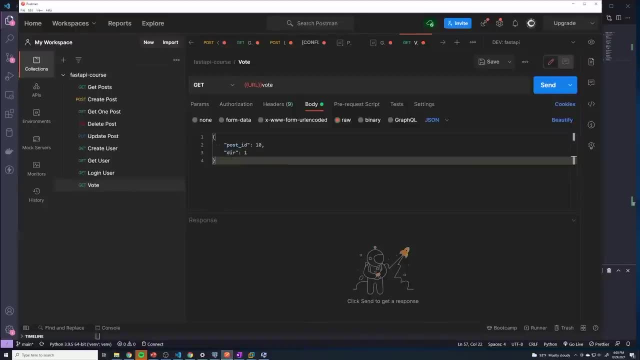 I actually forgot. Let's go to our schemas. Yeah, it's just der And this is going to be. let's see, let's there's gonna be a one so that we can actually like the post And remember this should be a post request. 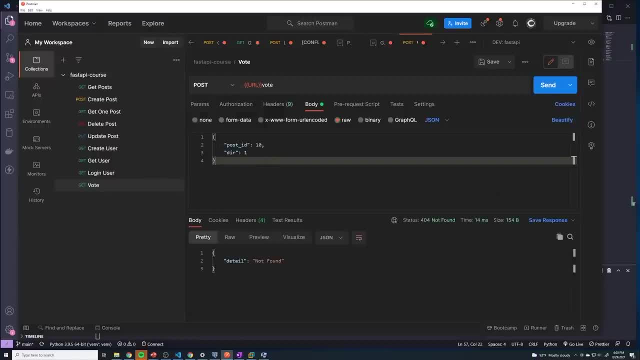 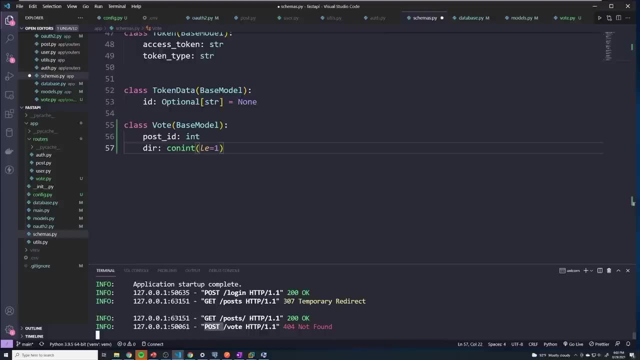 So let's try this out. Let's hit send And it looks like we ran into an issue. So let's check And it says that this specific route was not found And so that's obviously because we didn't- We didn't wire up this specific router. 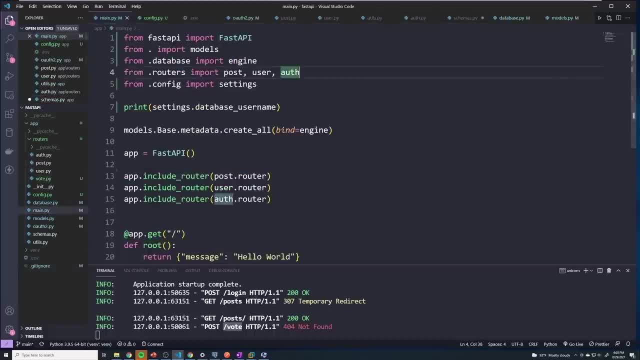 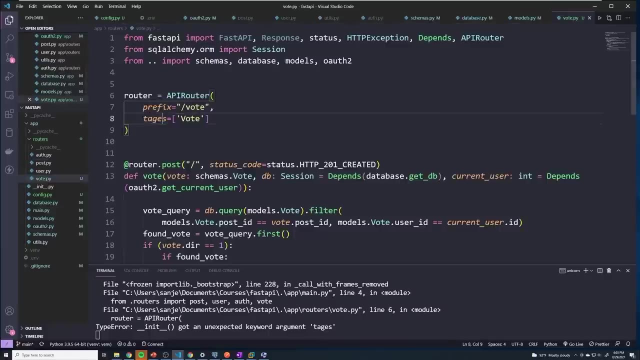 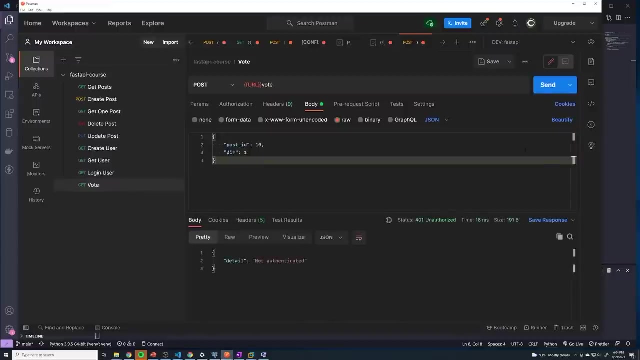 So let's go back to our mainpy And let's import vote, And then we can just copy this and wire up: voterouter Yep, And once again another typo. All right, let's give this a try now, So we'll hit send. 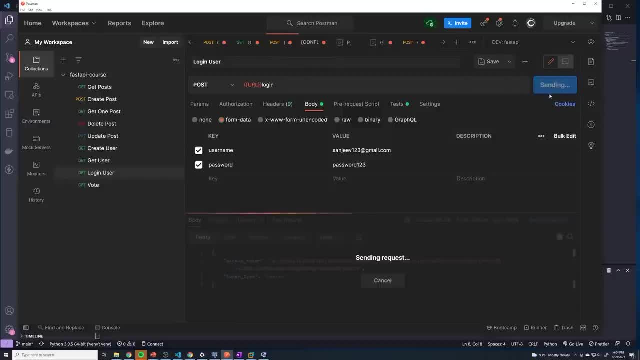 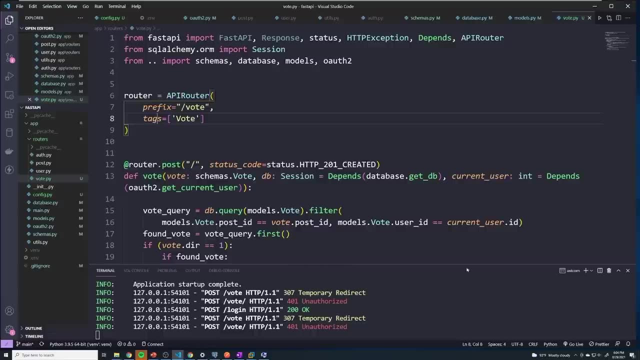 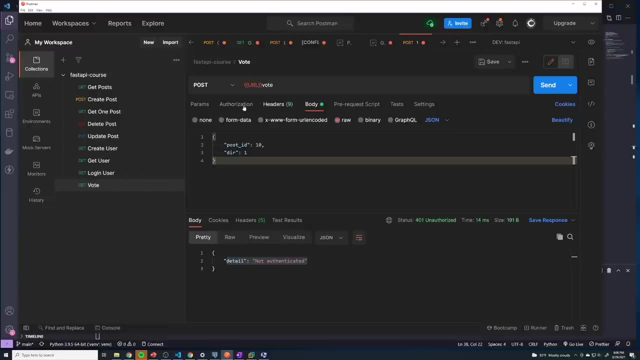 It says we're not authenticated, So let me log in Login user. All right, now let's try this. And it says that I'm still unauthenticated. And, guys, I realized why we're getting not authenticated. That's just because we have a new request and we have to make sure that we set the authorization. 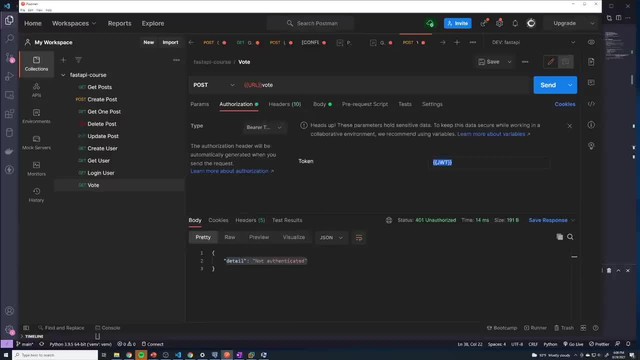 to be bearer token, And then we want to pass in our JWT variable, So it wasn't actually retrieving that. So now, if I try this, we can see that we successfully added vote. And you know, just make sure, Make sure that it actually did that. 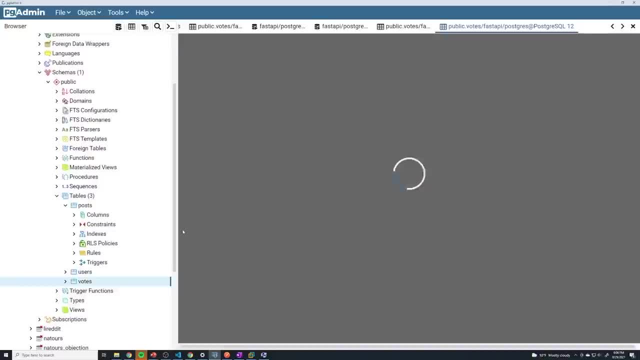 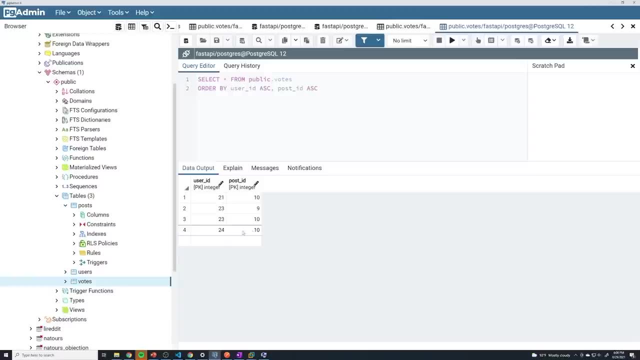 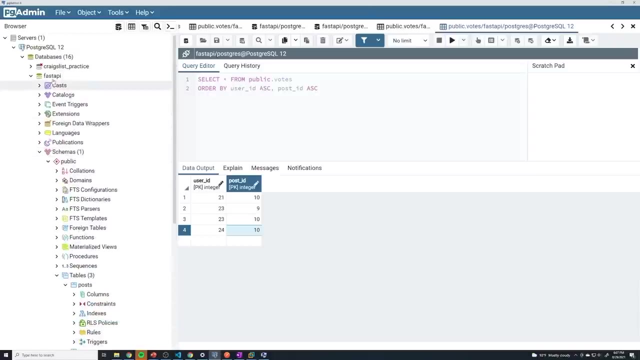 Let's actually go into our database and take a look at our votes table, And so we like to post, and it looks like I have some previous ones. So what I'm actually going to do is I'm going to delete everything from our votes table. 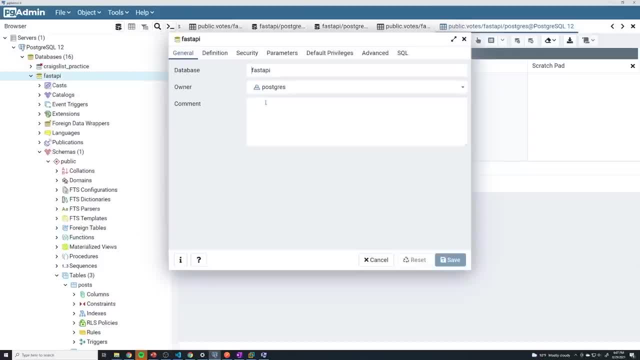 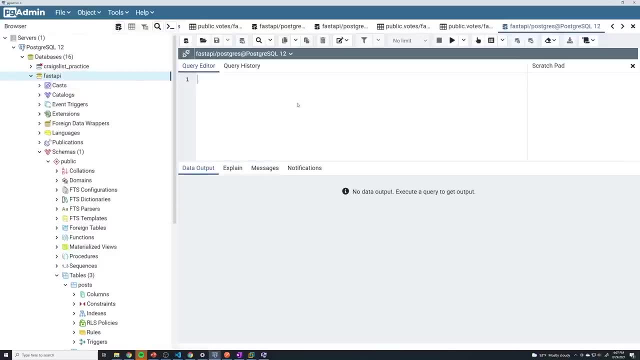 just so we can make sure it works, because I forgot who. I'm even logged in as. Let's go to properties. Sorry, Let me just do a query. I'm just going to say delete from votes. that's going to delete everything in our votes. 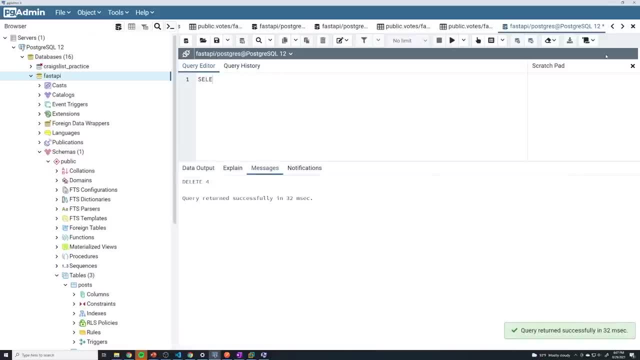 table, Perfect, And then we could just say: select from votes. We have nothing in there And let's try this again. All right, And so now run this. We can see that we did like post 10.. And I guess our ID is 25.. 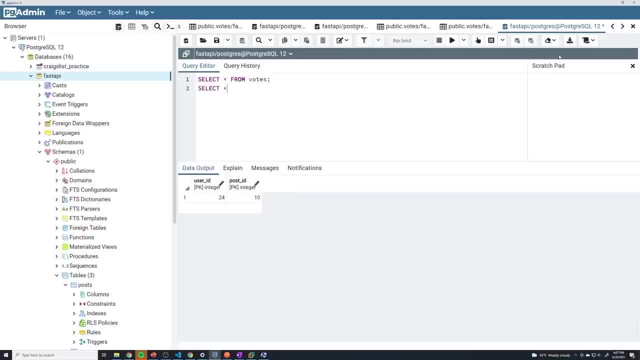 But we can just quickly verify that by: do select star from users, And I'm logged in as Sanjeev123 so we can see that that has an ID of 24.. So that works. Now what I'm going to do is: let's test to see what happens if I try to vote on a post. 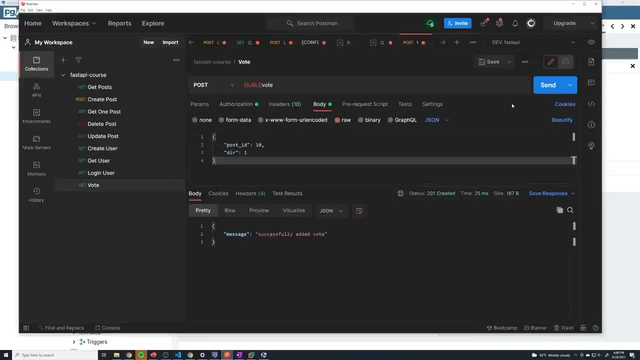 that I've already voted on, So I'm going to keep the vote direction to be one, And I know I've already voted on this post, So we should get user 24 has already voted on post 10.. Perfect, Now let's go and try to delete a post. 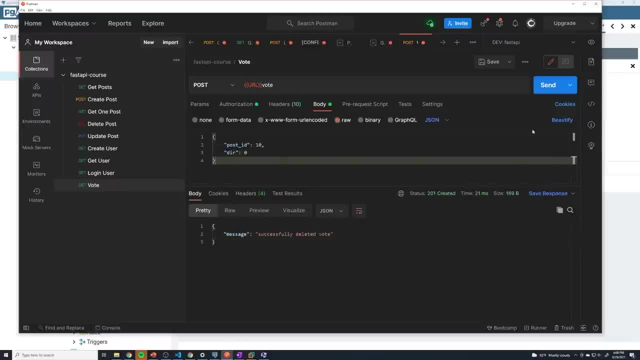 So I'm going to set the vote dir to be zero And let's see what happens. It says I successfully deleted the post or the vote And let's just do a quick query. We can see nothing is there And then if we try to delete a vote or a like that doesn't exist, we can see that vote does. 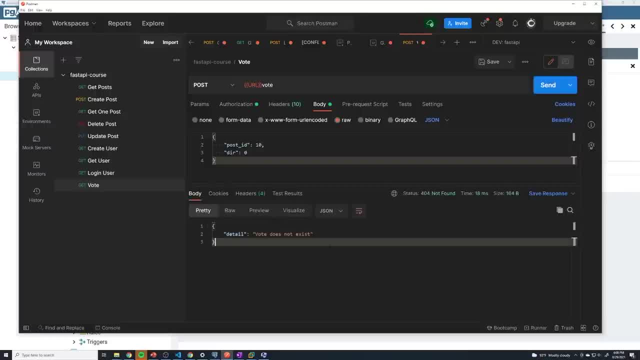 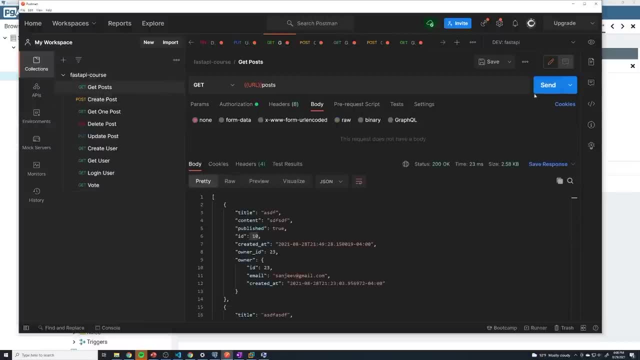 not exist. All right, guys, we've actually implemented all of the voting logic right there. The only other thing that we need to do is when we retrieve a post right, Whether it's through the get all posts or even a get one post. 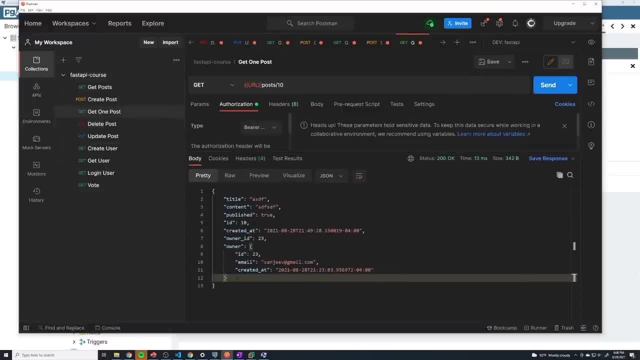 I want to have my fast API send the number of votes as a property, as a field here, so that you know when we load up posts on our front end application they can see the number of likes that a post has. that's usually how most applications work. 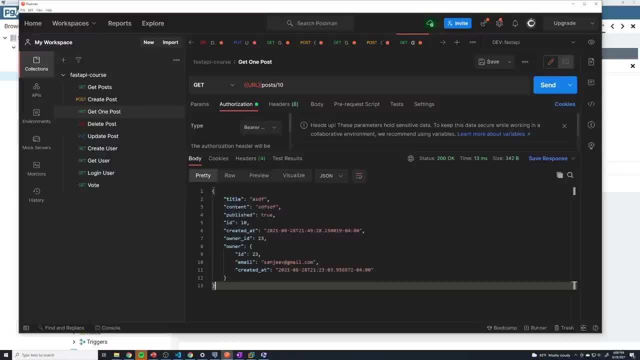 And I would like it to have it automatically send that information instead of having to send another query to our back end to see you know what is the total number of votes. I wanted to do It automatically anytime we retrieve any post, And that's going to be a little bit more complex. we're going to have to learn a little bit. 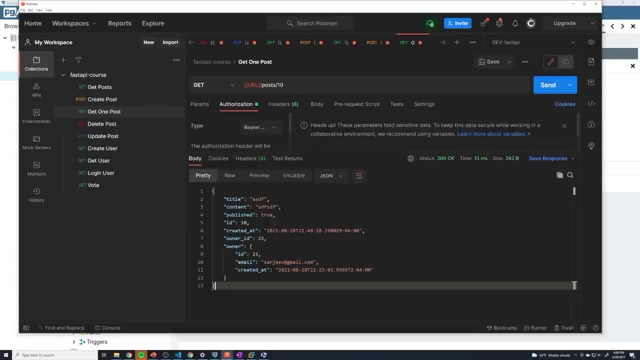 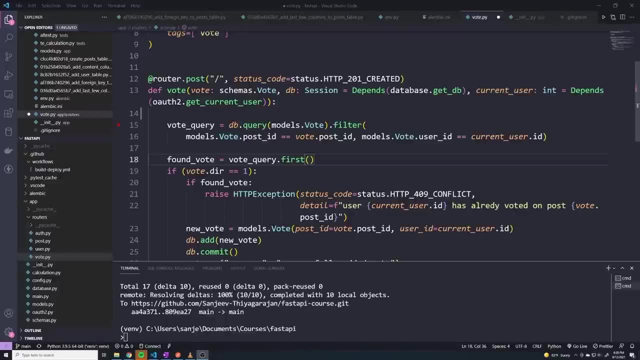 more about SQL, start digging into some of the weeds of SQL and Postgres And then, once we learn how to do it with regular SQL, we have to see if we can do this with SQL alchemy. After I finished recording all of the voting logic, or at least the router that handles- 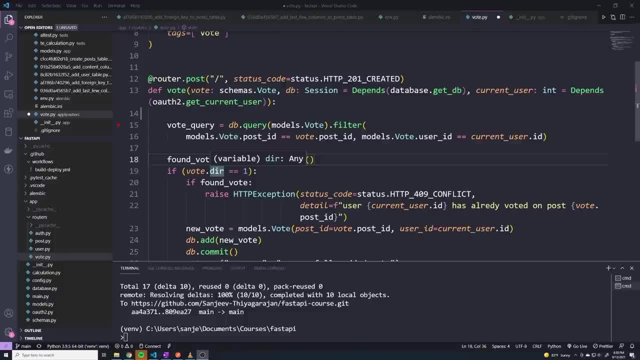 voting, I realized there's one tiny bug, And that is that right now there's no logic to actually detect if the user is trying to vote on a post that doesn't exist, Because if they want to vote on a post that doesn't exist, I want to ideally send a 404.. 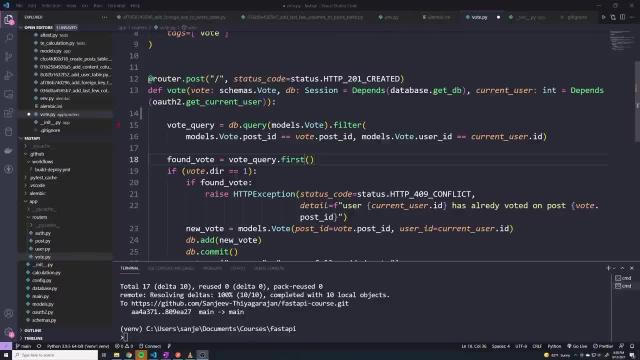 So what we're going to do is we're going to implement that logic, and it's going to be really simple. we're just going to query for the post based off of the ID first. if it doesn't exist, we're going to throw an exception. 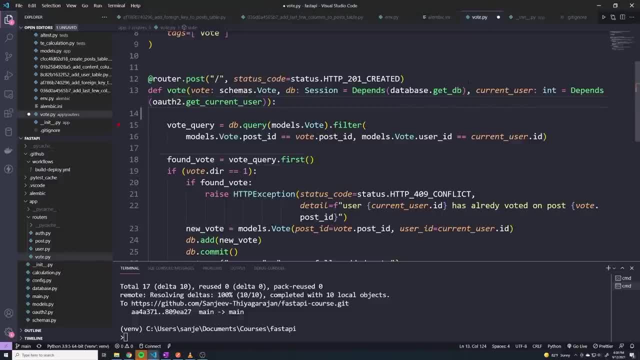 So, just like we've done with pretty much all of our other routers, whenever someone tries to access a post that they don't, that doesn't exist, then we're just going to simply send a 404.. So let's start off by making a query. 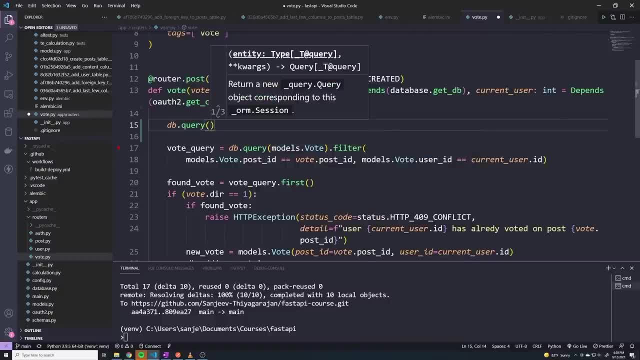 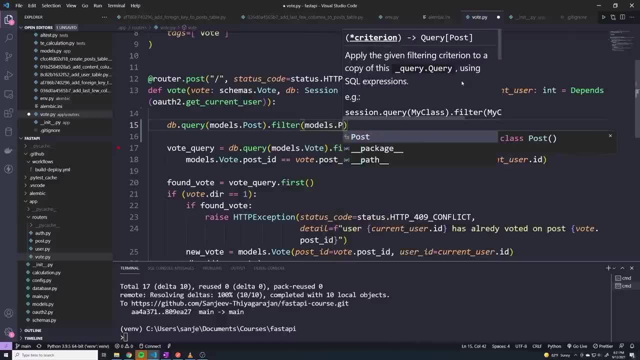 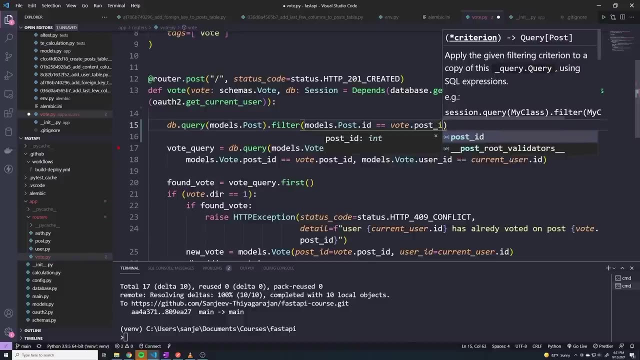 I'm going to do db dot query. we'll say models dot post And then what we're going to do is we're going to filter based off of the post ID. So we'll say models dot post. dot ID equals equals vote dot post. underscore ID. 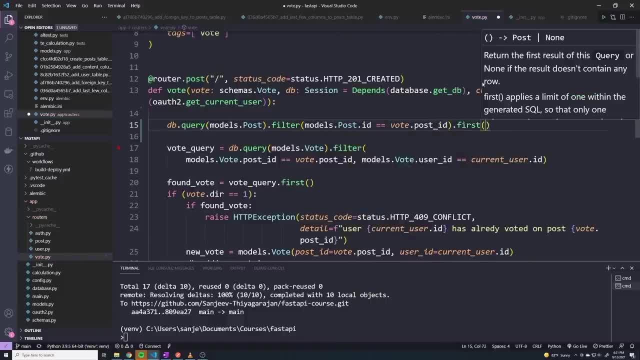 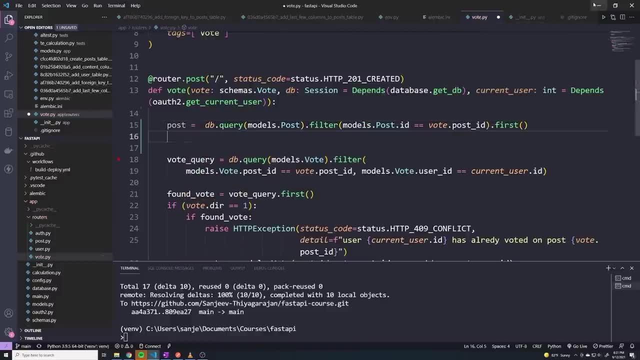 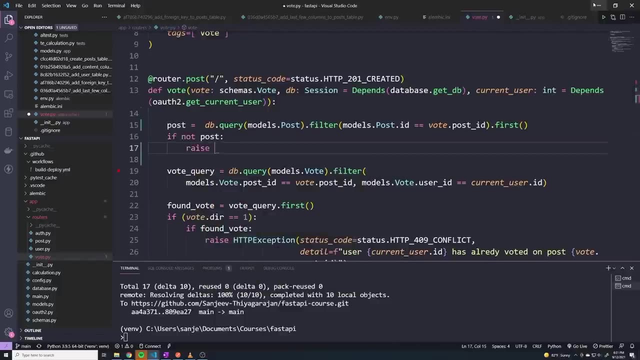 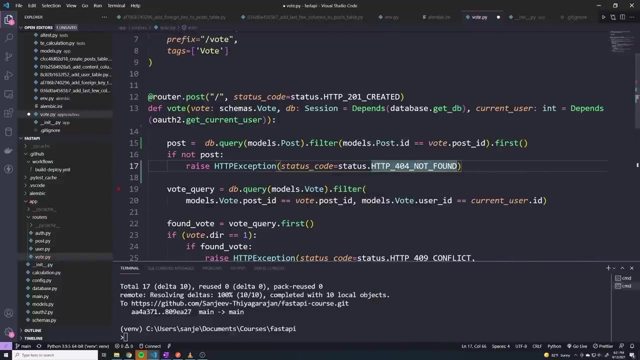 And then we're going to grab the first one And we'll save this in a variable called post. Then we'll say: if not post, so if the post doesn't exist, then we're going to raise an HTTP exception And the status code is going to be a 404.. 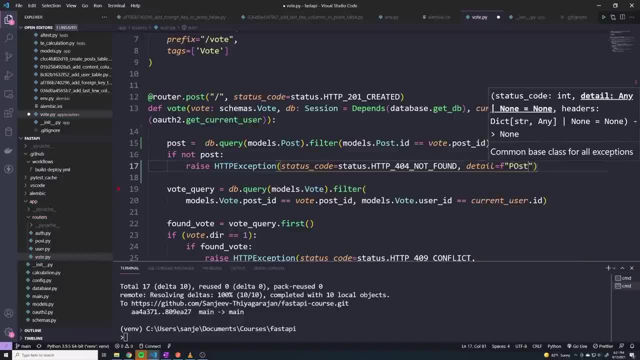 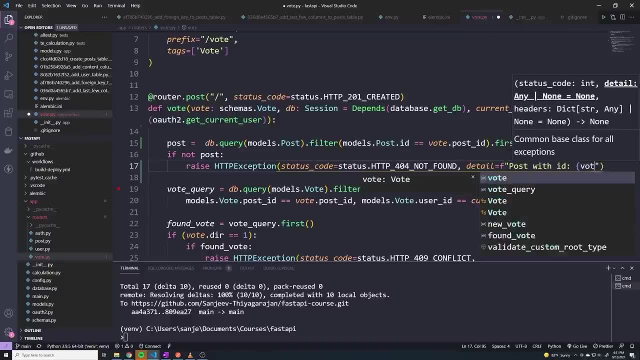 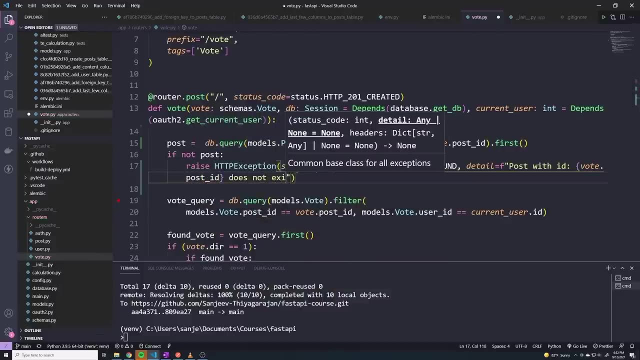 And the detail will be the usual F string that says post with ID and then we'll pass in. the ID Does not exist And that's all we have to do. And that's going to fix that little bit, that little tiny bug. 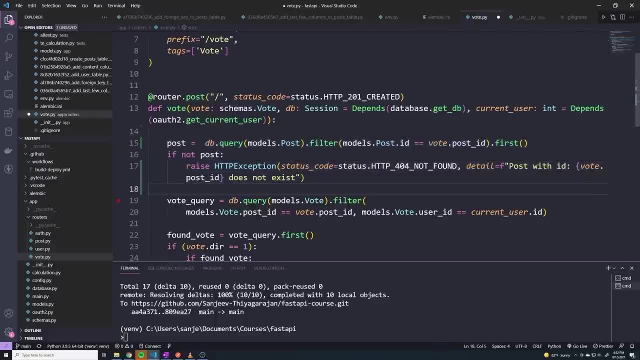 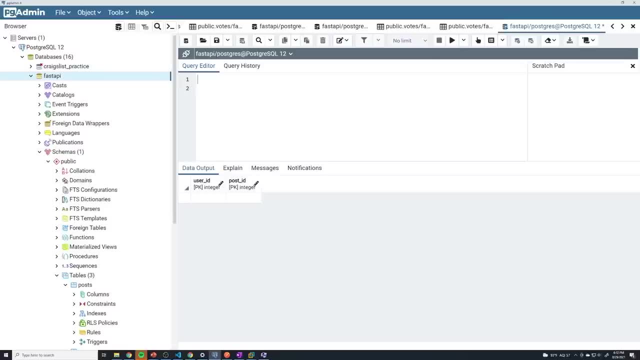 And you'll see that when we get to the testing section, we can now test to see if the post doesn't exist as well. Up till now, we've been working with very simple queries. we've just been querying a single table. However, now that we have more than one table and all of these tables have built out their 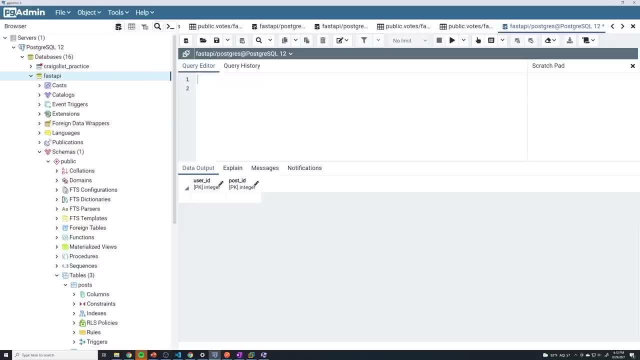 these relationships. you're going to see that eventually you want to be able to get information from two tables at the same exact time, And this gets a little complicated. But the way we actually do that is by using something called a join. So we join two tables together And, as an example, 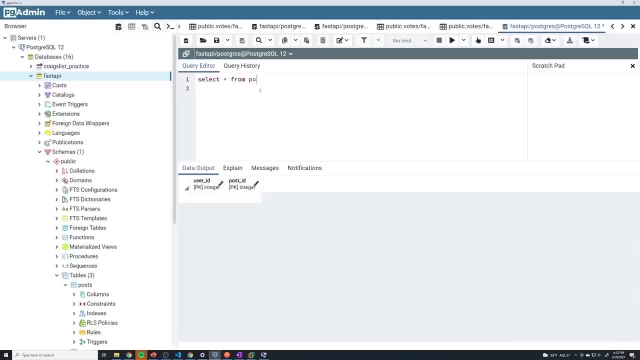 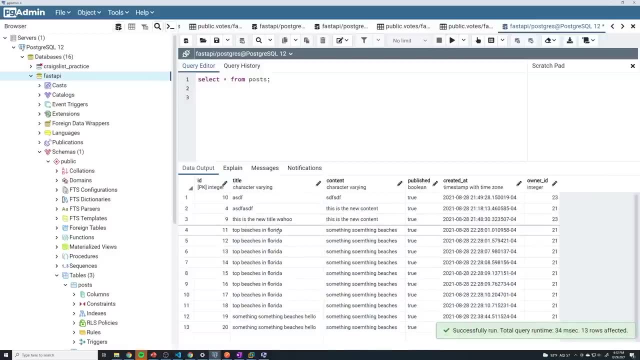 let's say I want to get all of my posts, So I do a select star from posts. That's great and all. However, you know when we're sending back the, the posts, to the user right, the, or our front end. our front end has no idea what a owner ID of 23 is. he doesn't know. 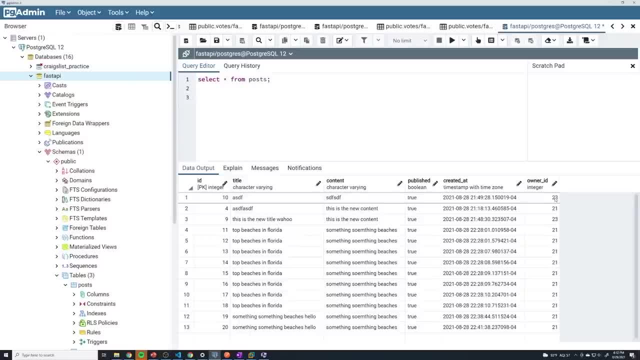 what that is, And we ultimately want to display the username or the email of the user that created that post on our front end. So what we would have to do- if we can only, you know, retrieve data from one table at a time- is we'd have to then individually go and then fetch all of these users. 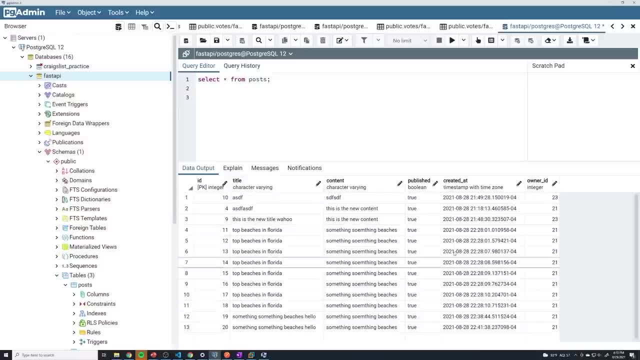 from the user table one by one so that we can actually get the email or the username. And that's a little inefficient Having to do multiple queries. if you ever get a chance to, it's better to just do a single query. 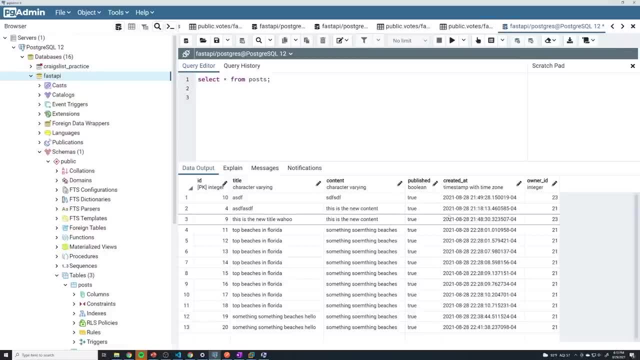 and get all of the pieces of information that you're interested in. So I'm going to show you guys how we can join information from two tables, because I would also like to get all of the user information based off of the owner ID field, that's on the posts table. So how do we do that? Well, 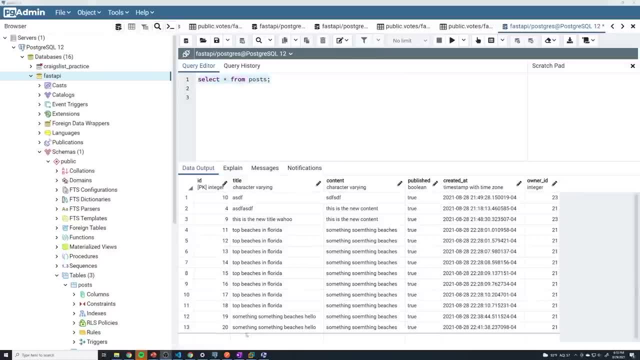 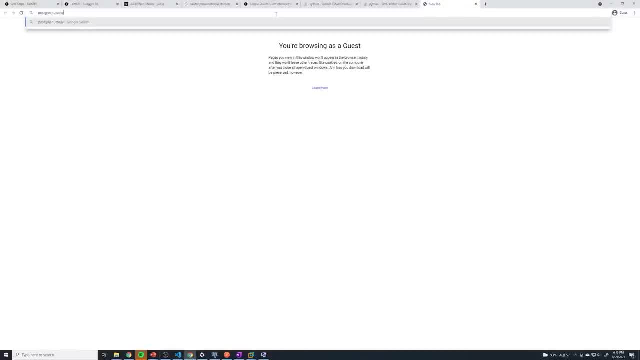 we start off a query just like this, And actually, before we go into this, what I would like to do is show you one of my favorite websites. So if you go to post grass tutorial, just search for that in Google. you'll see that there's a website called postgresql. 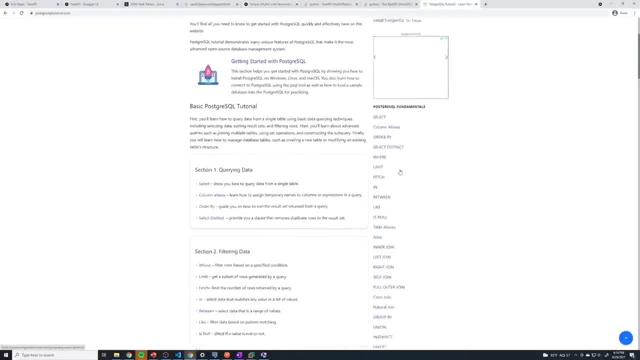 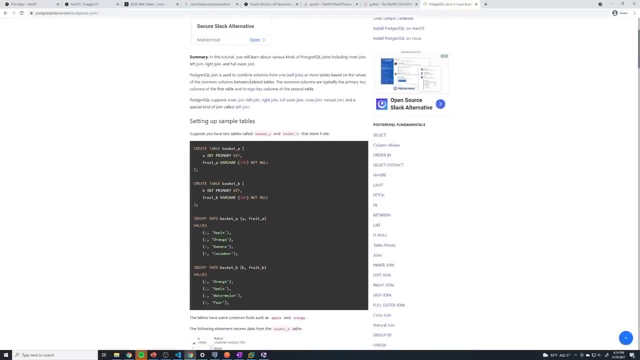 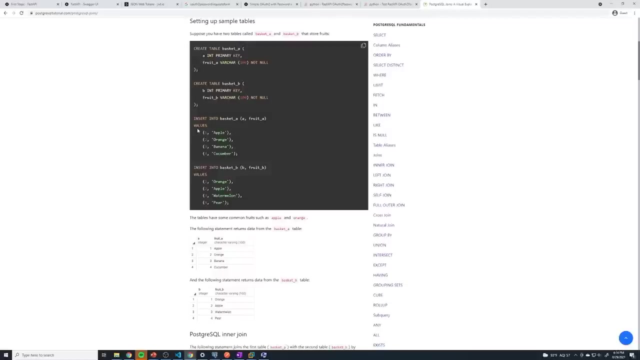 tutorialcom. This is one of my favorite sites And I want you to go to joins right here. So this is how we get information from two different tables And this, this page. you does an absolute marvelous job of explaining how to actually join two tables And it goes over the different types. 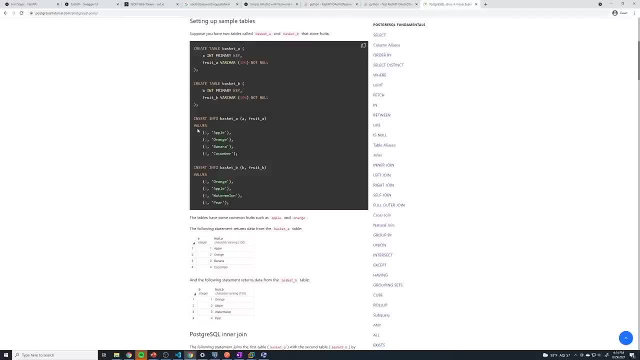 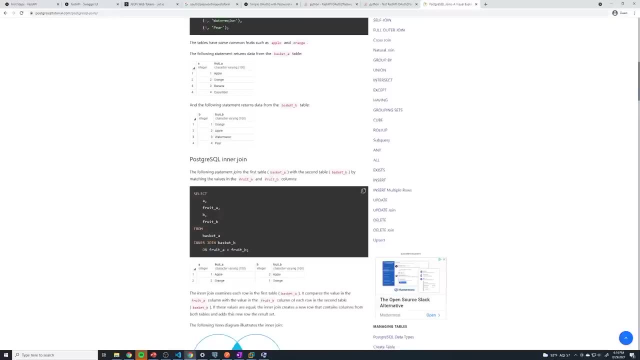 of joins, because there isn't just one method. You've got left joins, you have inner joins, you got outer joins, you got right joins And I strongly suggest you guys quickly just kind of read through this just to get an idea, Because I don't want to cover every single join, I'm just going to show you the ones that we need. 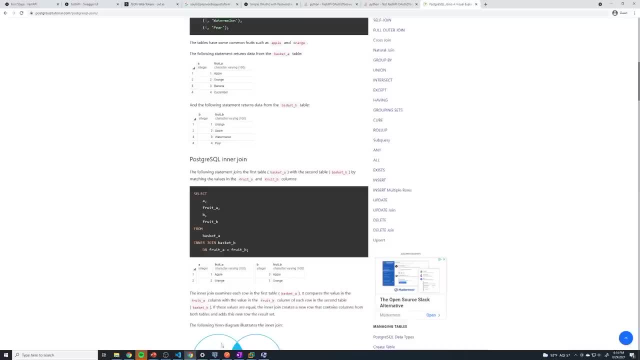 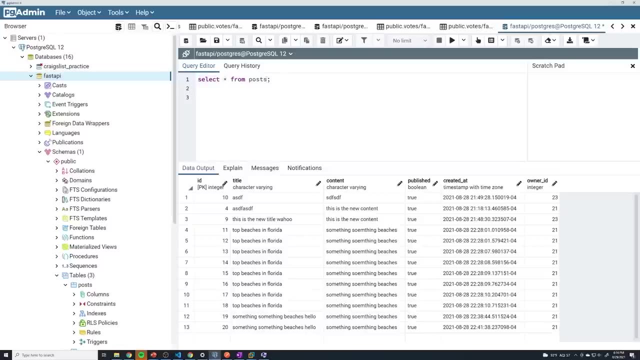 to get the data that we're interested in. So let's go back to Postgres And let's create our first join. So here I'm, do select, I'm just grabbing all of the fields And I'm going to grab it from. 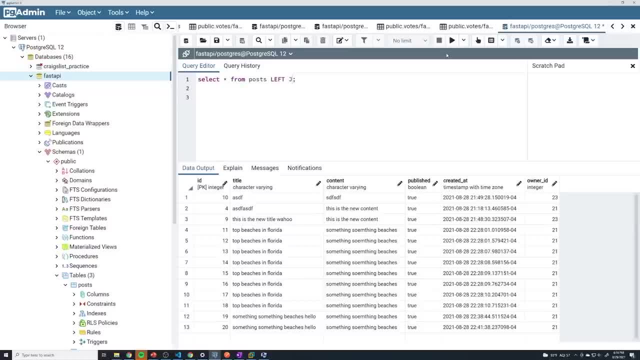 the post table And what we can do is I can say left join And then we specify the other table we want to jam into my query. So now I want to get data from the users table, So I do users And then we have to find a field in both tables that 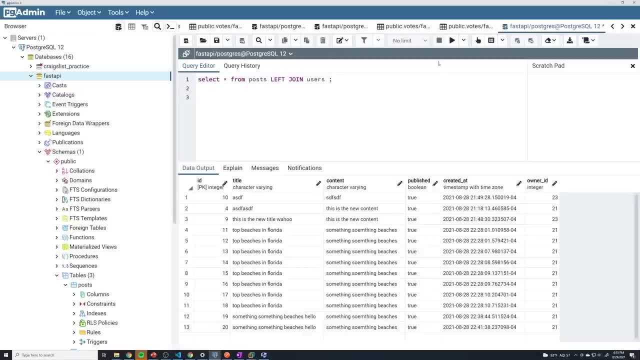 we need to match on or join the table on, And since we want to find the specific user associated with the person who created this post, we need to join on the owner ID. So what we say is on. so this is how we specify what it should join on And we want to say we grab the first table's. 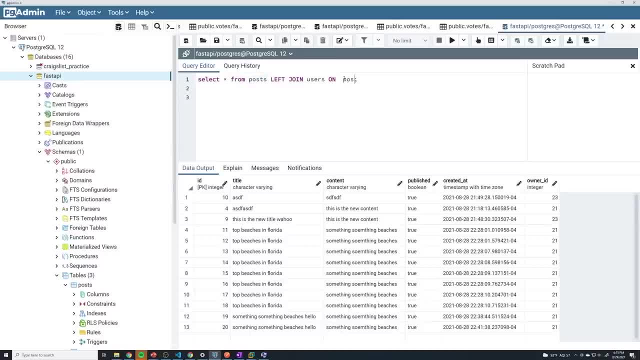 name right, the posts table. we grab posts And then we say dot and then we grab the specific column we want to join on, So owner underscore ID, And then we just say it equals two. And then we grab the second table, which is called users, And then we grab the specific column from the 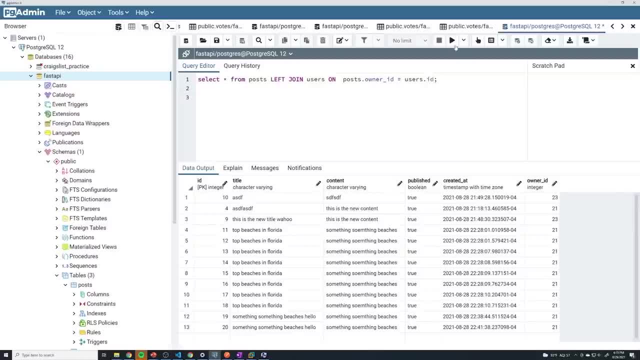 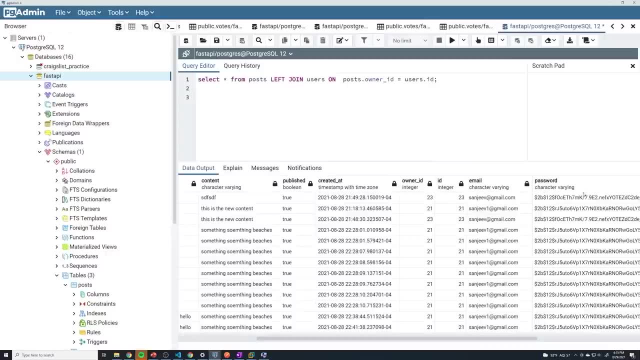 users table we want to join on, which is usersid. So now, if I run this- take a look at that- it took all of the user data And it jammed it right into one single query with the posts, And so now I get. 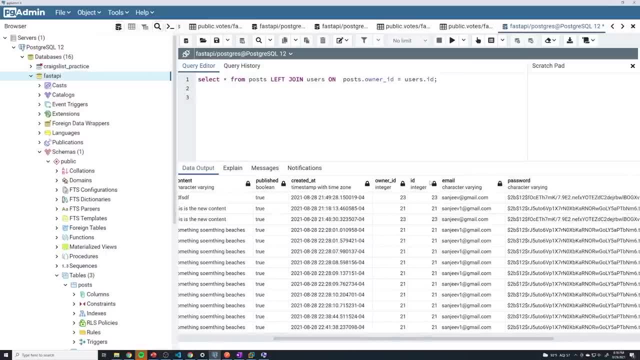 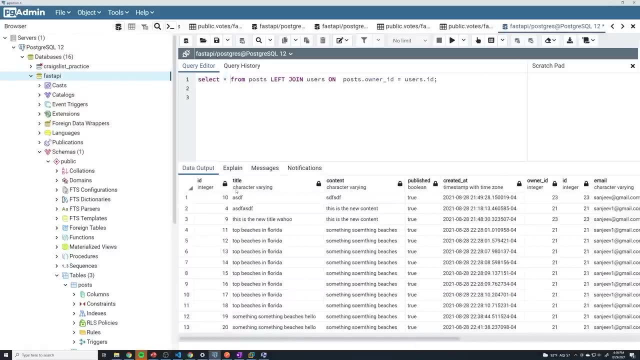 the entire post And I also get information about the specific user because we joined on owner ID and the user ID together. So it was able to kind of take that information from the other table and match it right up to here Because we did a star. it's going to grab the columns from. it's going to 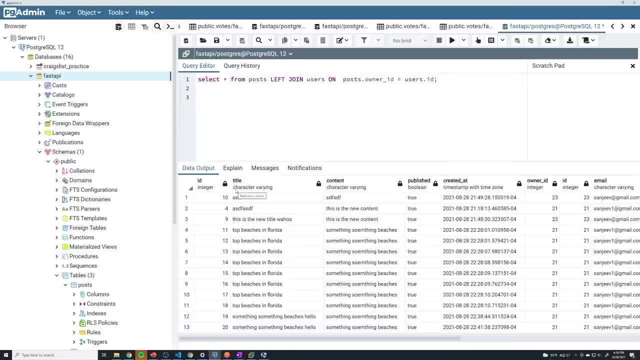 grab every single column from every single, from both of the tables. And there may be times where maybe you don't want that, maybe we just want a couple of columns. So let's say we want the title column, Maybe we want content And maybe we want email- Right, and this should allow us to grab the title which comes. 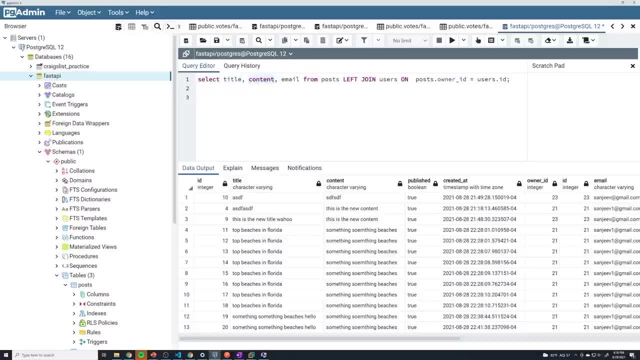 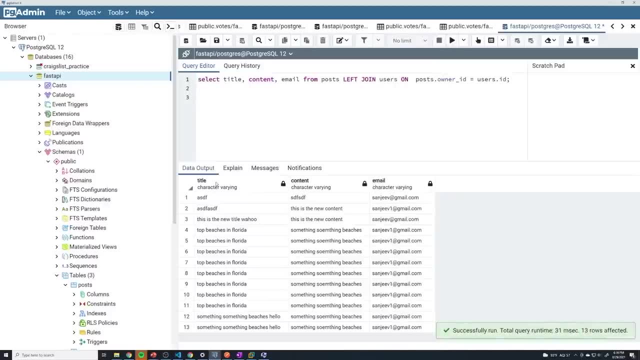 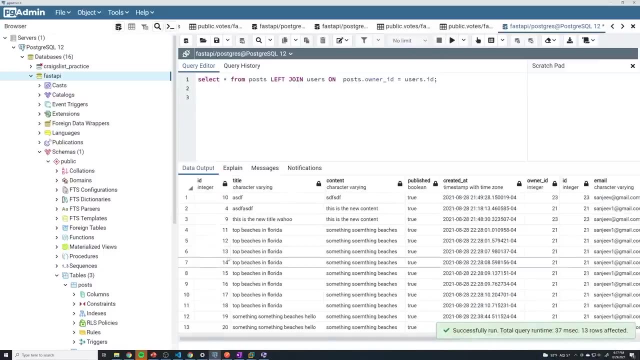 from the post table and the content which comes from the post table and then email which comes from the user table. So let's see what happens when I run this Right. you can see I got the title, content and email. Now if I remove this and go back to everything, just real quick, let's say 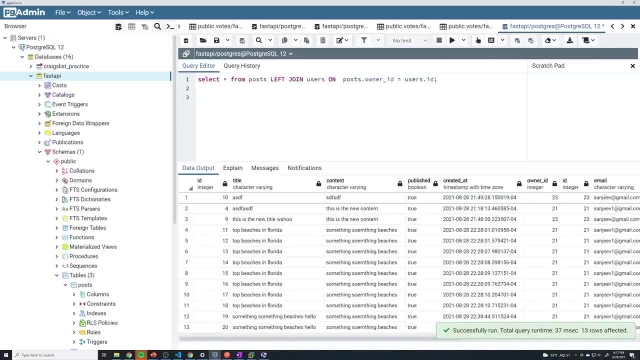 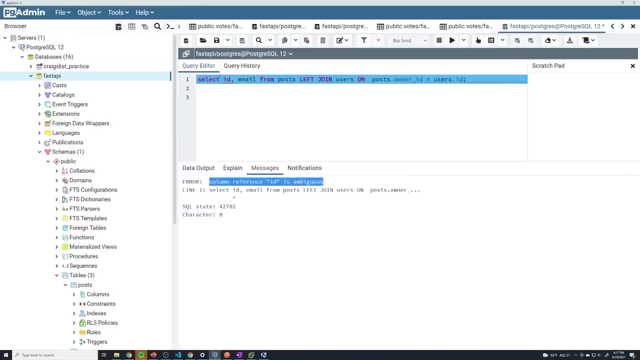 I want to get the post ID and the email. Well, let's see what happens. I'm going to do ID and then email. Well, it looks like we have an error. It says column reference ID is ambiguous. So what exactly is happening here? Well, I'm going to remove this and show you exactly what happened. The problem: 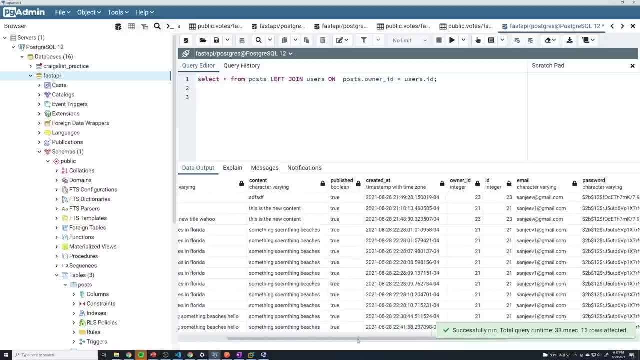 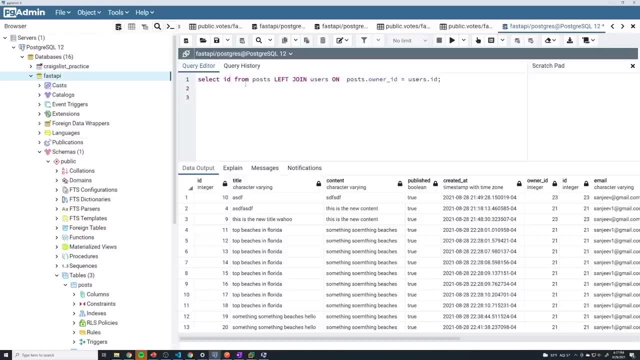 is is that the post table has a column called ID And the user table has a column called ID. So when I just say ID, it has no idea which column I want. So that's why it's saying it's ambiguous. So what we need to do is, anytime there's potential for confusion, we always have to specify the table. 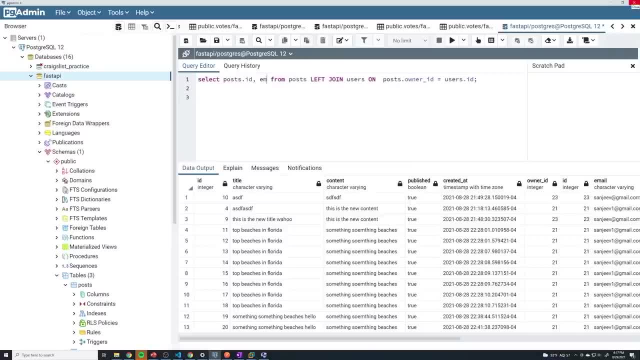 name before, so I can say postsid And then I can say email. Now I don't have to say: you know, user dot email, because only the users table has an email column. However, if there was an email column in the post table as well, then we would have to append the table name first, So you only 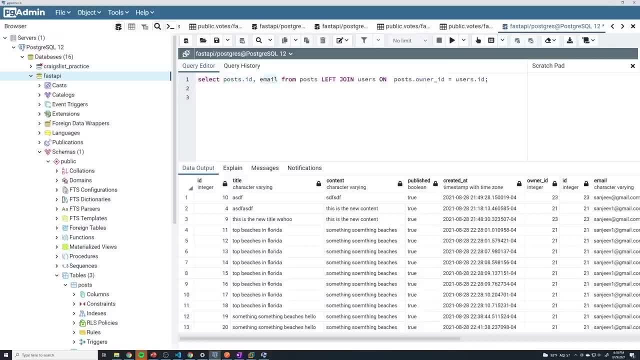 need to do this when there's confusion. However, if you want to just kind of stick to a certain convention, you can just set up every single property to have the table name beforehand, so that you know which table it's coming from. makes it a little bit easier to read, And so now I got. 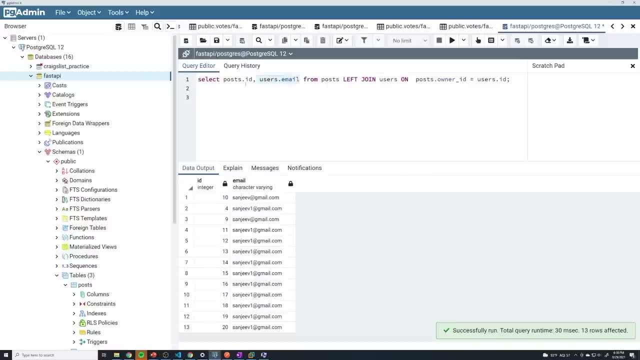 just the ID and the email. Now let's say I want to get every field from one of the tables. I can say posts dot star. that's going to grab every field, So it's grabbing the post table. And then the star means Hey, grab every single column. And so I could do that. it's going to grab everything from the post. 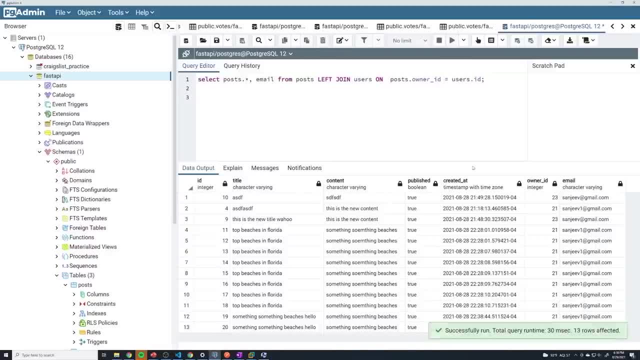 table and then I can grab maybe just the email in this case, And so this kind of ultimately does what we had wanted it to do, Because you know, I told you guys, we want to be able to get the email or the username information for each and every single post. And if we want to, you know we can. 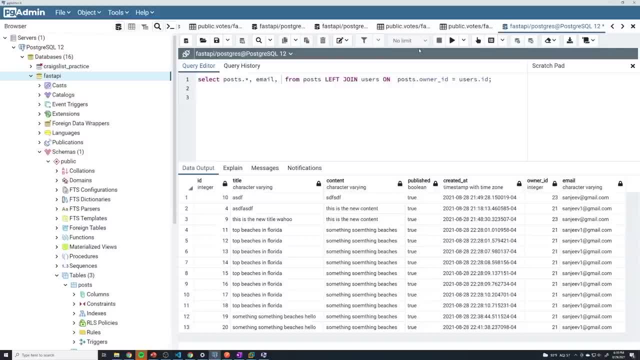 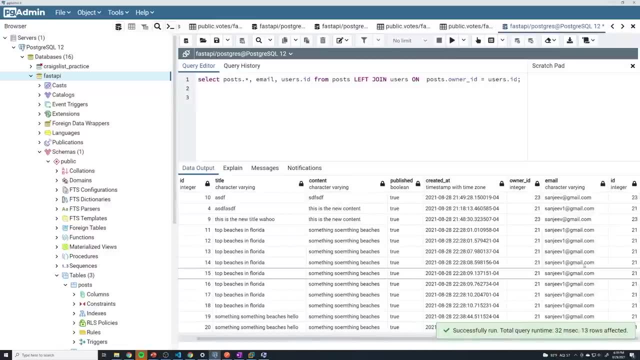 add in some of the other fields, maybe the, maybe the userid, So the user ID. however, that's just going to match up with the owner ID, but just to show you guys, there is some flexibility And, as I mentioned before, 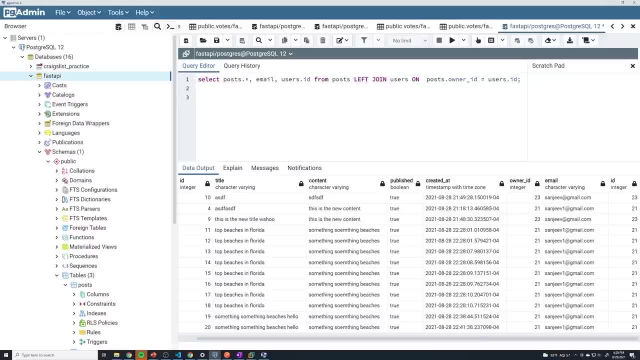 are different types of joins. There's left join, there's right join, inner join, outer join. I don't want to spend too much on it, but I do want to cover just a few things. All right, so the direction references which table. So right now we're working with two tables. There's the first. 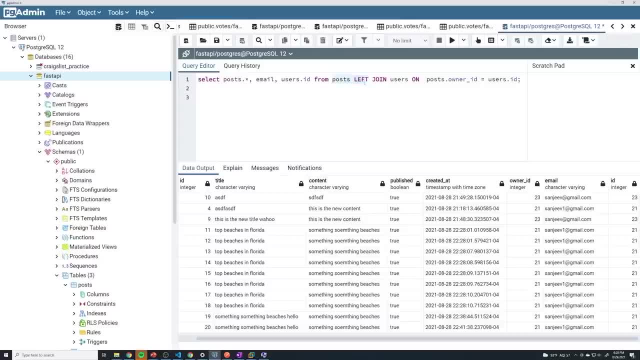 table that's referenced by from and then the name of the table, And then there's the second table, which is referenced after the join, which is right here, And so the first table that's referenced is always referred to as the left table And the table on the right the second. 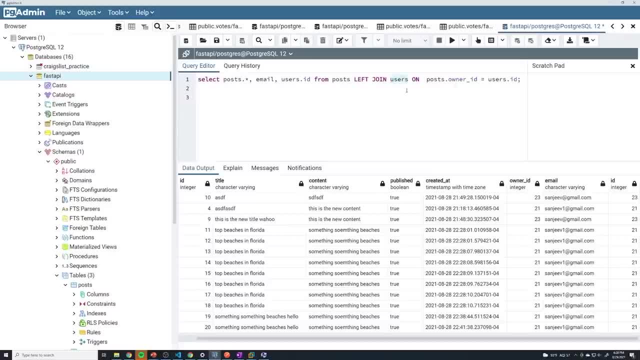 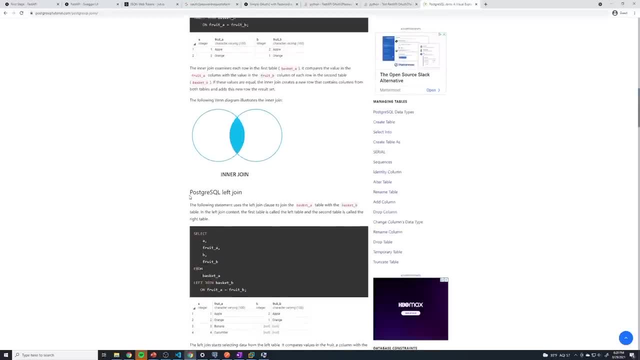 table that's mentioned is always going to be the right table. So you got the left table and the right table, And so when we do join, what it's actually doing is well, I think this page actually gives us the best explanation. So a left join select data from the left table, And I don't know. 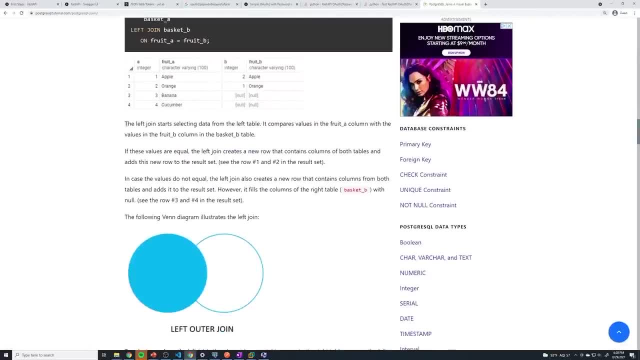 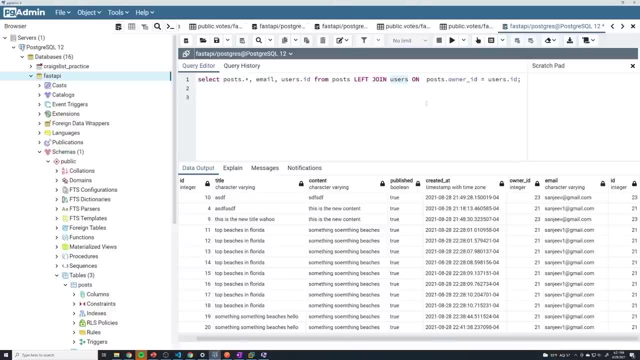 if this is big enough for you guys, but I'll zoom in. So it's going to select data from the left table, it's going to compare the values between the two columns that we have selected And for us, in this case, it's going to be post out owner ID on the left side. 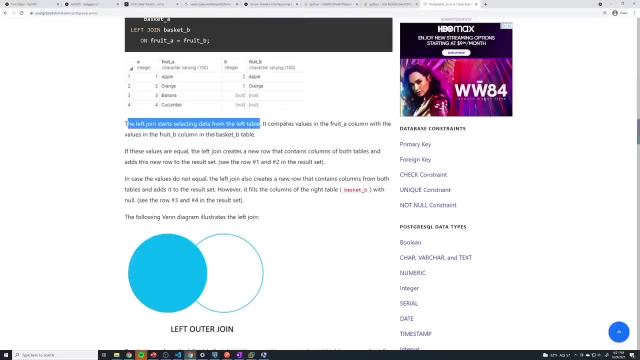 And then usersid on the right side And it's going to find where those values match And if they are equal, the left one creates a new row that contains the columns of both tables and adds this row to the result set. And what's important is, in case the value does not equal, the left join. 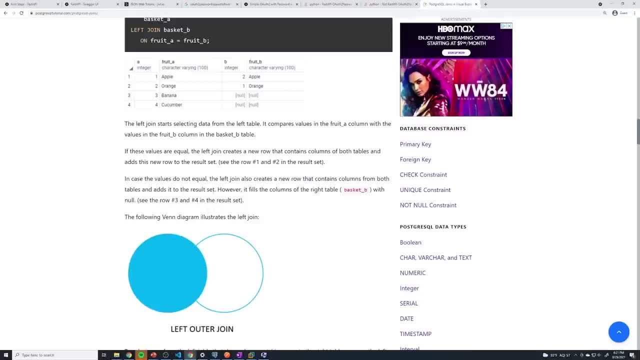 also creates a new row that contains the column from both tables and adds it to the result set. However, on the right side, the, the value is going to be set to null. So if we ever had a post that didn't have a value, we're going to have a new row that contains the columns of both tables And if 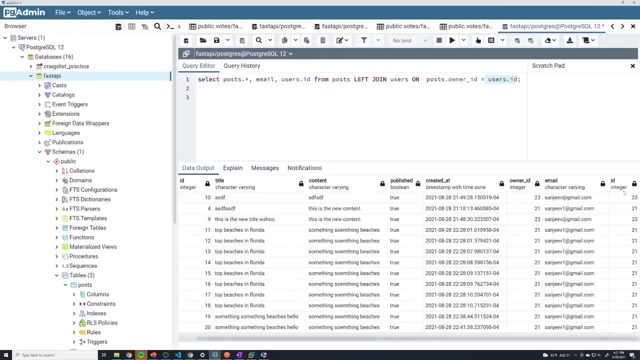 we ever had a post that didn't have an owner ID, then what would happen is we would see the- the user information- all set to null in that case, or the email would be set to null. However, since the way we set up our table is that every single post must have a owner ID, we're never going to run. 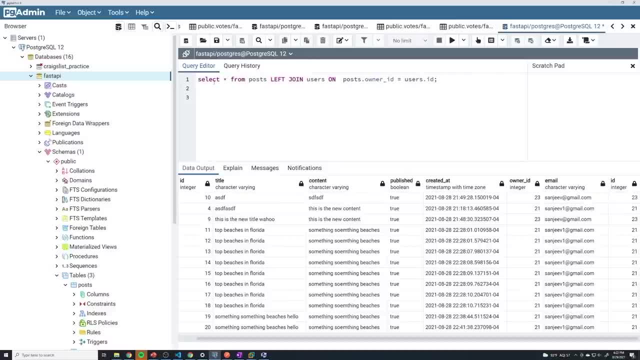 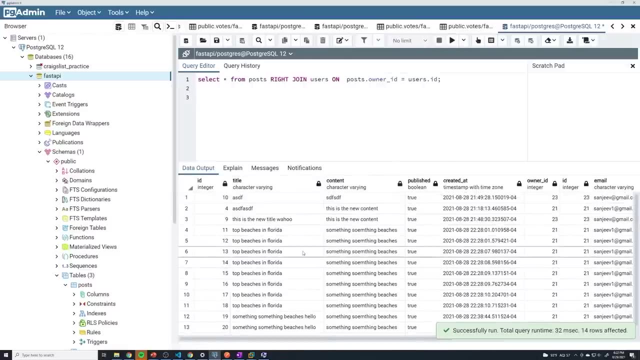 into that situation Now, before we move any further, just to show you, guys, what a right join is. it's the exact same thing, but in the opposite direction, And so let's take a look. look, And things look a little bit different now, Because what's happening is that we're going to 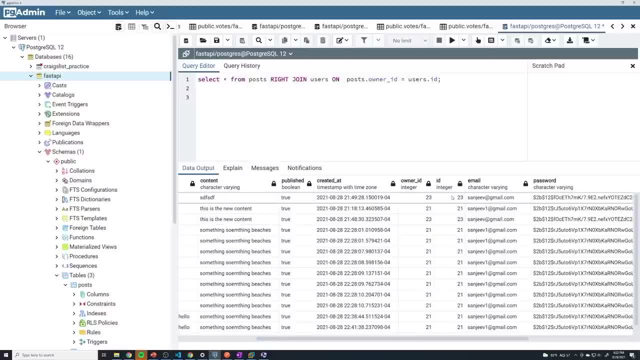 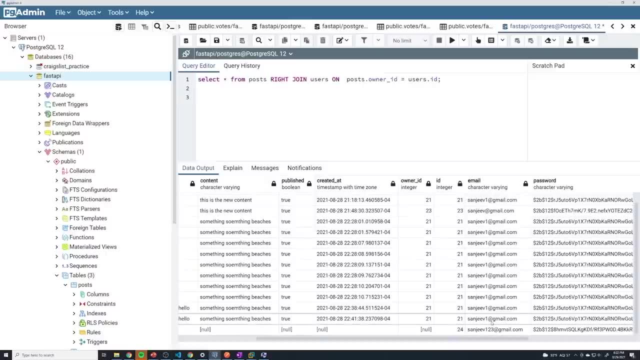 is that we're going to go through the two tables and find if the owner and the owner ID and the ID of the user match And we're going to join it on that, And we're going to do this for every single entry And then at the end you can see that user 24 has no information on the left side. 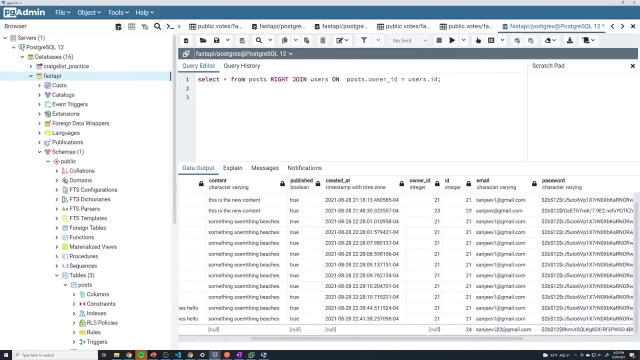 And that's because user 24 didn't create any posts. So the right join will show you instances where something exists in the right table but it doesn't exist on the left table. The left join will show you something that exists in the left table but doesn't necessarily exist on the right. 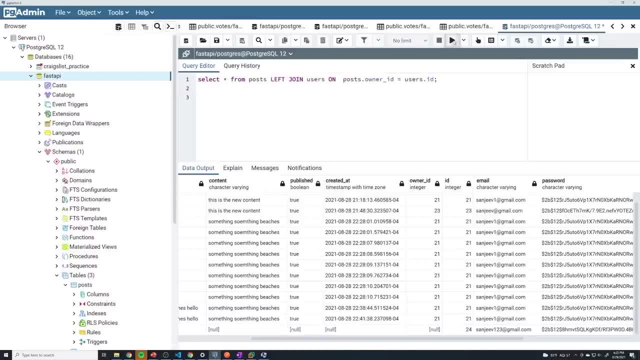 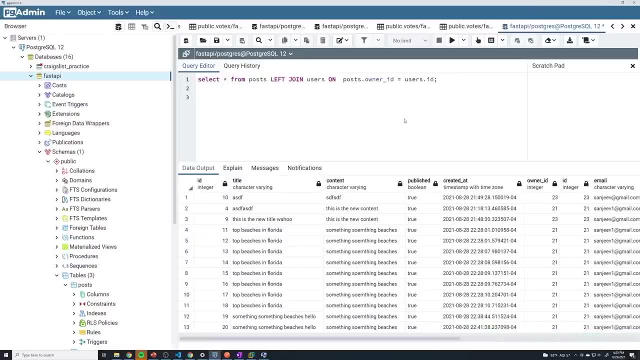 table. But I'm going to change this back to left join. And now what I would like to do is: it would be great if we can get the number of posts by each user right. How many posts has each user created? So is there a way to do that? Well, there is actually. 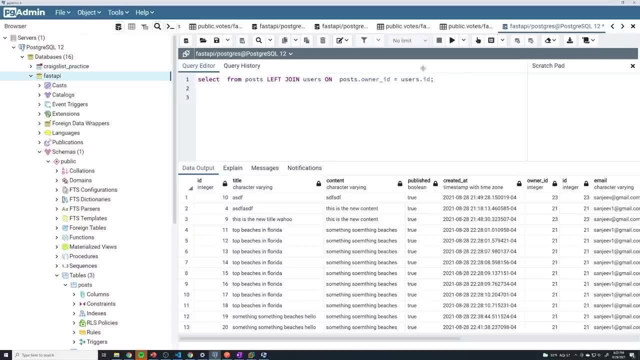 So what I'm going to do here is I'm going to grab the users dot email, actually users dot ID, and maybe we want the users dot email as well. Actually, we'll just get the ID, And here at the end I'm going to say: I want to group by 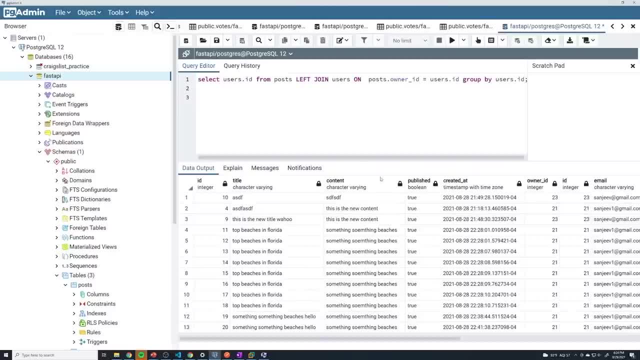 users dot ID. So we're going to find all of these- So that's the Default ID, all of these entries in our join, and then group them based off of the user ID field from the user column. And so once we group them, we can then actually count up all of. 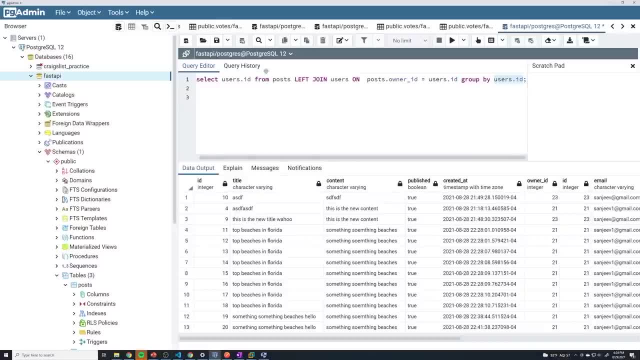 the columns- Sorry, all of the entries on a per user basis. So if I say user ID and then we say we can use a builtin Postgres function, And here if I put in star- and I'll come back and explain what this means- we can hit run and we can. 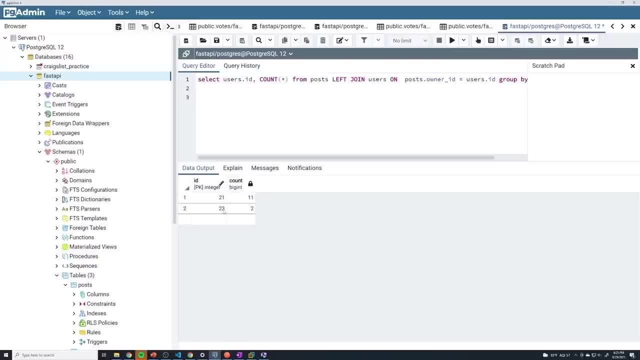 see that the user with an idea of 21 has 11 posts and the user with an ID of 23 has two posts. The only issue is if I actually do another query right here and do select star from users. there's actually three users right And one of. 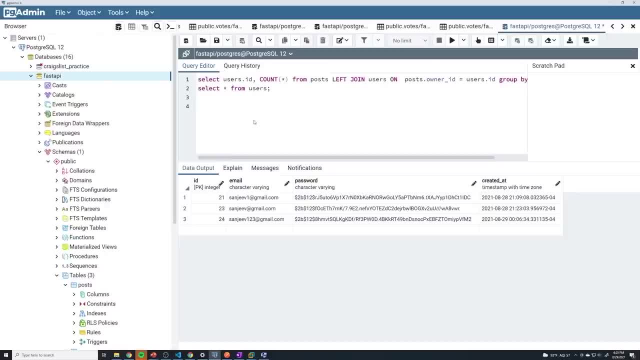 them hasn't made any posts And so that's why we don't see it in that list. And if we want to be able to see it in that list, we need to actually change our query And, like I mentioned, the right join. if I actually remove the account column right here and we just do a star, this is going. 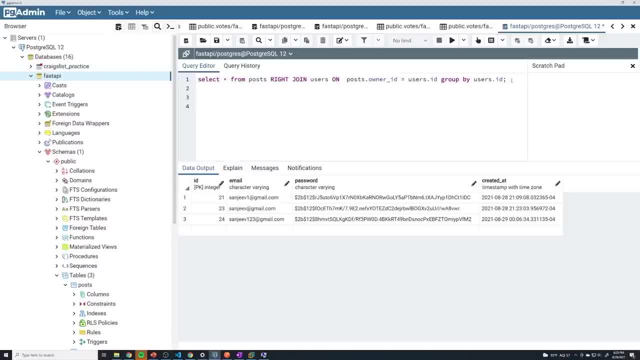 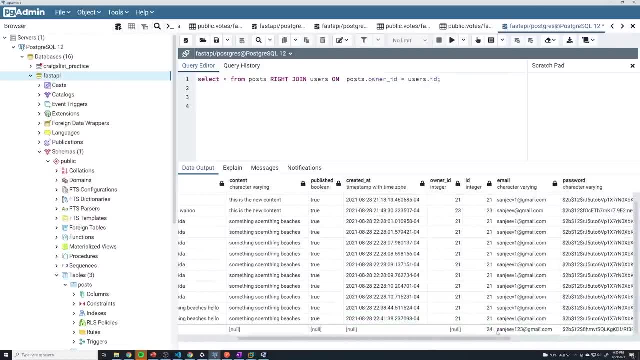 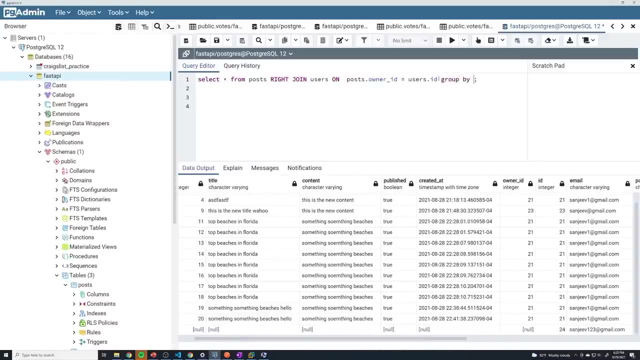 to actually list every single user, even if the user has no posts. And so if I remove the group by ID, real quick, right, you could see down here I have user 24 with no posts. that's exactly what we want. And so now I can say: group by users, dot ID. And then here I'm going to say: 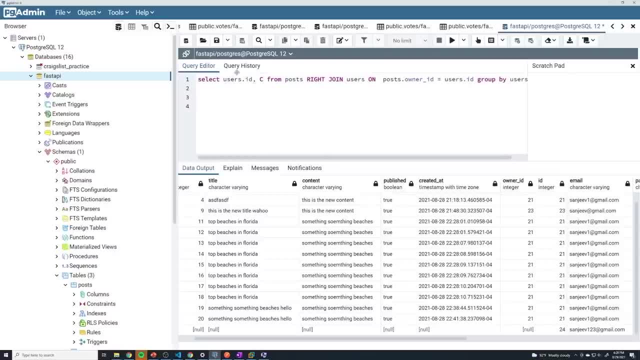 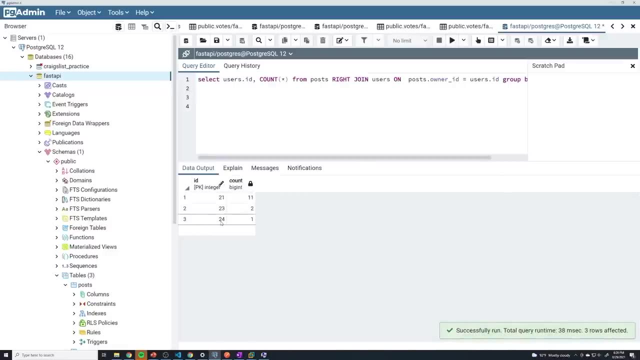 select users dot ID And then we grab the count. So let's see if this works And notice how all of the post fields are completely empty. So that's, that's perfectly fine, And then we can run this And you can see that it seems to have worked right. User 21 has. 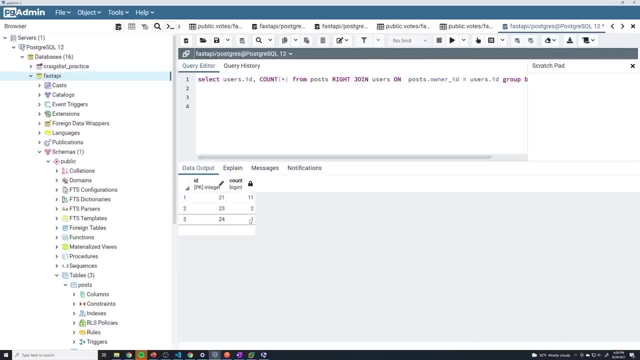 11 posts. user 23 has two posts and then we got user 24.. But it says that there's a value of one, And the reason for that is that when you do star right here, that means it's not a post, And then you can see that it's not a post, And then you can see that. 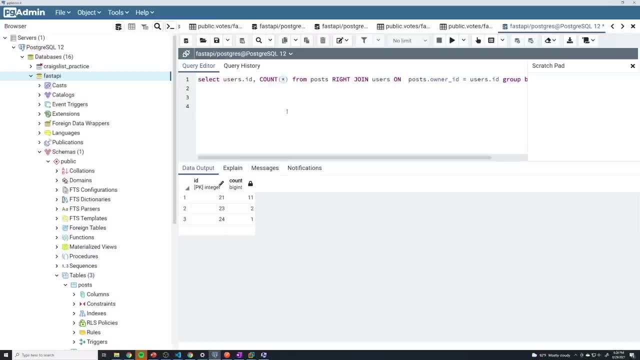 it's going to count null entries. So, since we have that one null entry, it's going to count that as one. So instead, what we're going to do is we can actually pass in the name of a column And so, once again, I'm actually going to copy this, paste it into here. we're going to remove. 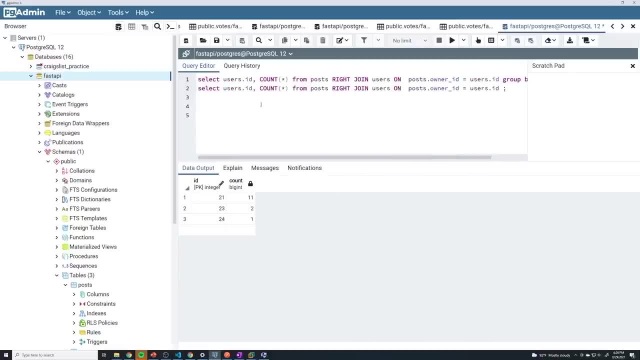 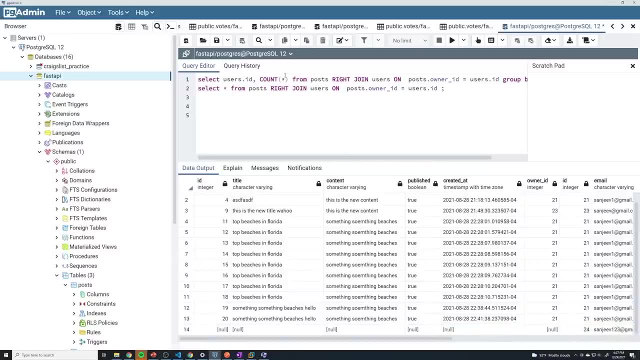 the group by and then just do a star. So we're going to get every entry. except because we did count star, it always ends up counting this as one. So you- that user 24, is always going to have one entry, but that's not accurate because he doesn't actually have any. 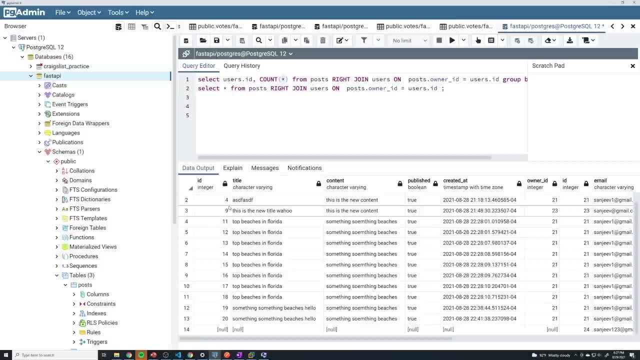 So instead of doing count star, we can actually pass in a column that we want to count, And so in this case we can pick any of the posts column that we're trying to retrieve, And so I can just say post dot ID, And so when you pass in a column name, it does not count columns that have a null. 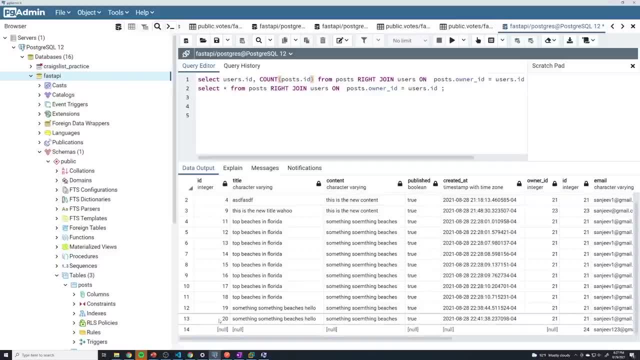 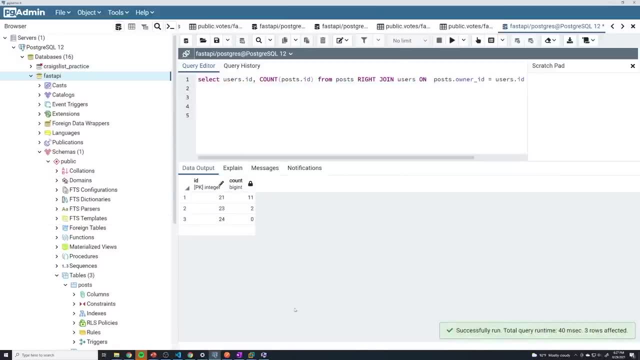 value. So if the user doesn't have any posts, he won't have anything under post dot ID, And then if I just remove this query and then run this, it's going to have any of the posts that we're trying to retrieve. So if I just remove this, you can see that now I have successfully gotten. 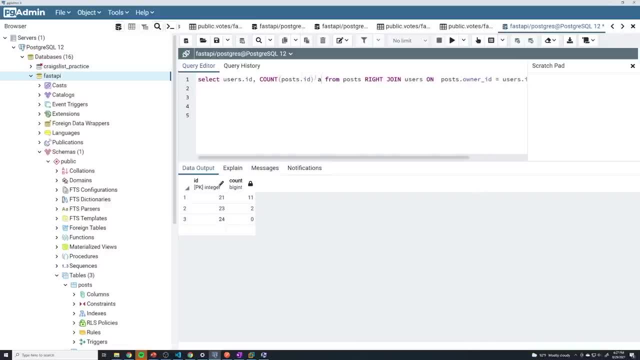 the exact query that I want, And I can rename this column as user underscore, post, underscore, count or something that's a little bit more readable, And then you know I can grab any other field that I want. Maybe I also want the users dot email, And so that way we get just 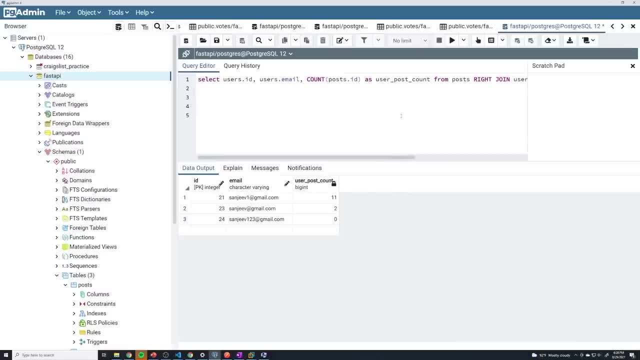 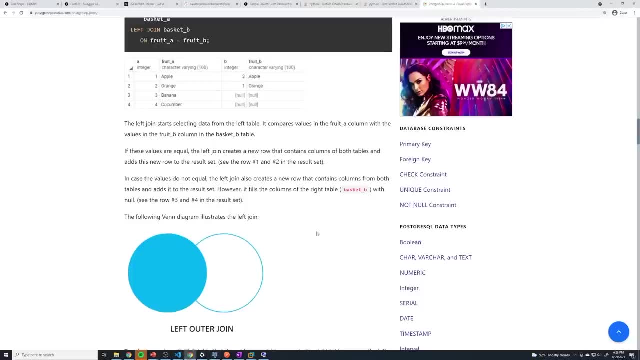 the information that we ultimately want. So you can see that doing these queries, they do get a little bit more complex and you have to practice this a lot, And so I definitely recommend you actually just read through this document, set up a few example tables and just practice doing your. 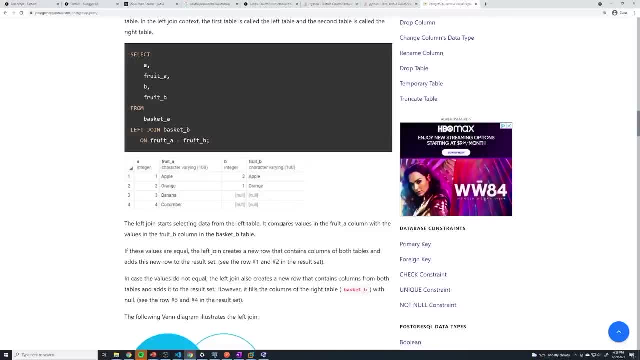 queries, But we're going to spend just a little bit more time on these queries so that we can figure out how to get the total number of votes. It is a little bit longer of a process, but I want to make sure that you guys understand exactly what we're doing. Alright, guys? so let's move on to. 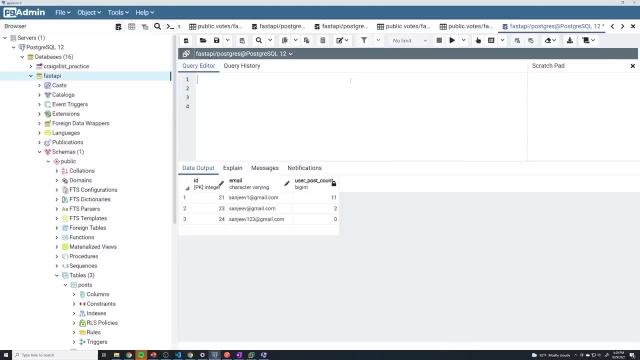 working with our posts table and our votes table. So I'm going to do a join on those two. So let's start off by doing select, And then we're going to go ahead and hit save, And then we're going to do select, And then we'll just do star for now And we'll say select, star from, And then in this, 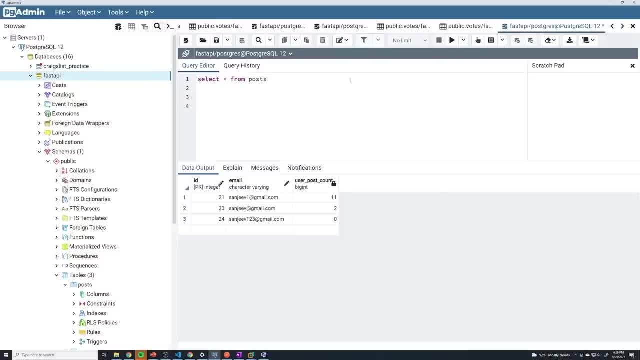 case posts. And keep in mind, guys, I mentioned that the first table you reference is the left table and the second table that you reference is the right table. It doesn't actually matter which one is the left or right. The only thing that matters is that you set up the right direction. 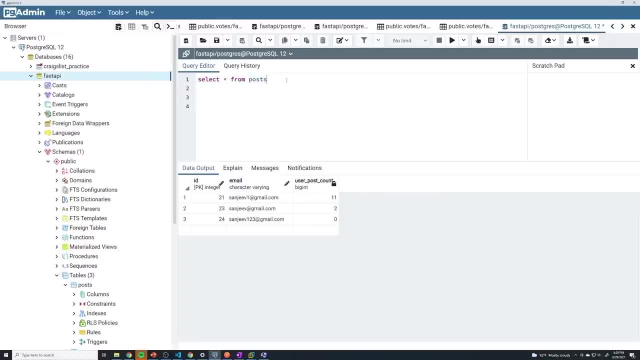 of the join. So if we set up posts as the left table and we want to do a left join, then if we ever rewrite our SQL query and set up our our votes table to be the left table instead, then we just have to flip the join to be a right join. So it doesn't matter which table comes first. Keep. 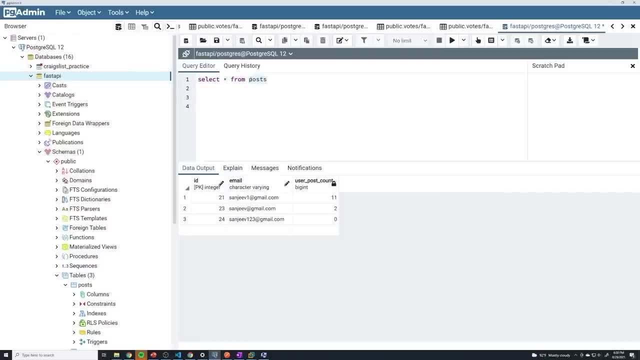 that in mind, So you don't have to start your query on just the posts. You could do this on votes as well, And you just change the direction of the join. But I like to do posts And then we're going to try a left join once again And we'll say that the other tables can be votes. 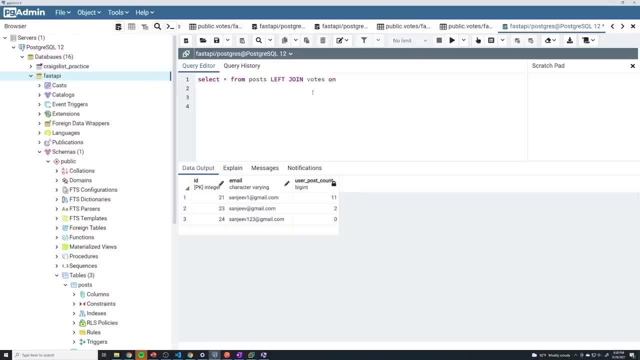 and we're going to join on. Well, if we take a look at our votes table- which I'm actually just going to cut this out real quick And save that in my scratchpad- I'm going to just say select star from votes. We'll run that Right. so there's going to be a user ID and a post ID And then, if 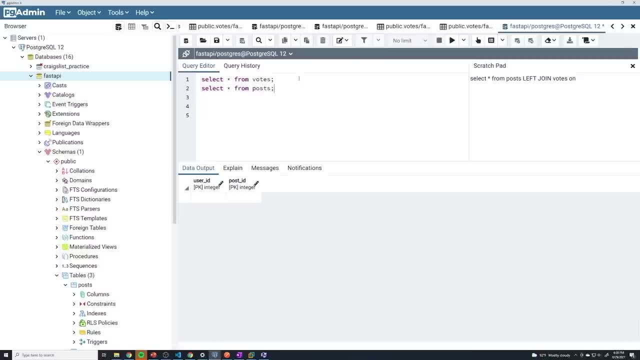 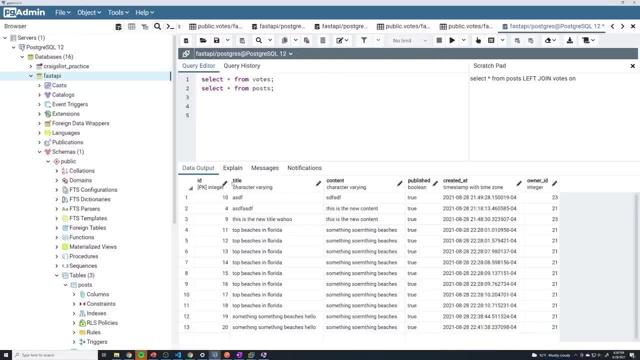 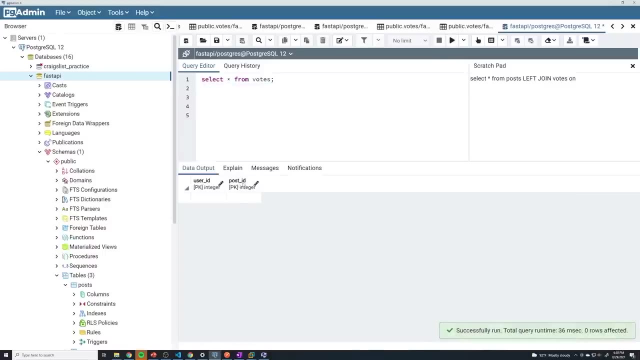 I do a select star from posts. we have all these fields So I think you guys can guess the exact column that we need to join on. So we need to join on post that ID and then votes dot dot post underscore ID. So whenever those match we need to get a result. So I'm going to go into. 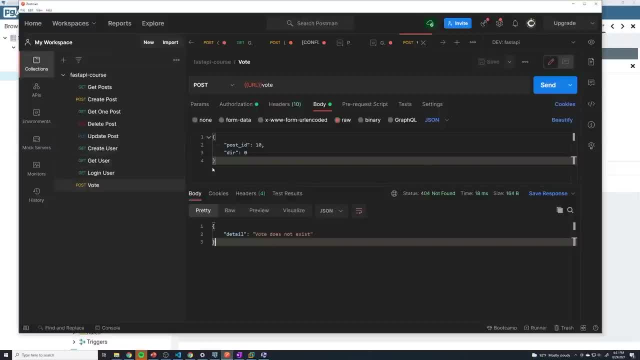 my application and just run a few. I'm just going to vote on a few posts so that we actually have some data. So I'm logged in as a user and I'm going to vote on post 10.. All right, we successfully. 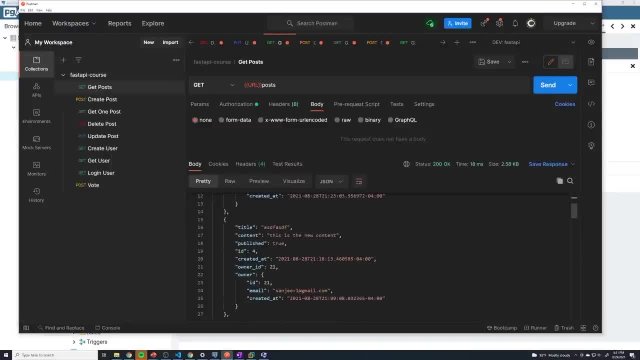 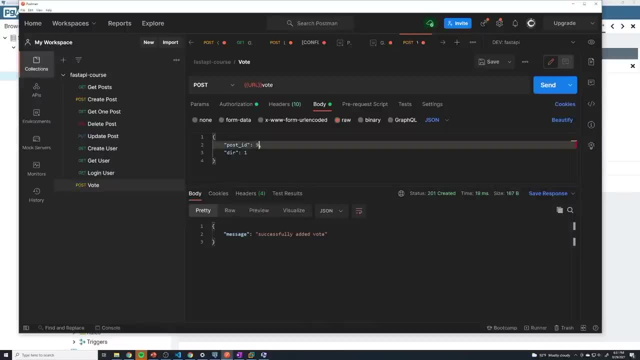 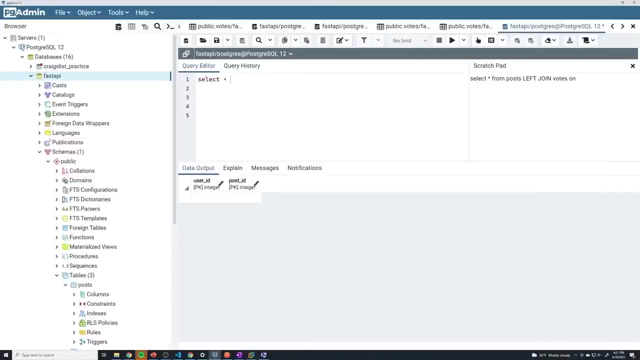 added votes. I'm going to get a whole bunch of other posts. I'm going to vote on post four and nine, Alright, and I'm gonna log in as a different user. Now Let's see who else I got. Alright, I'll just login as Sanjeev, I guess. 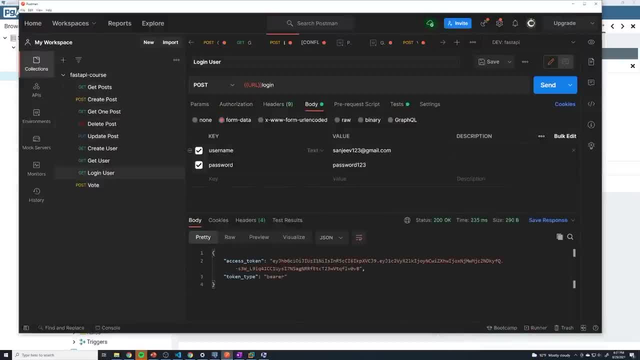 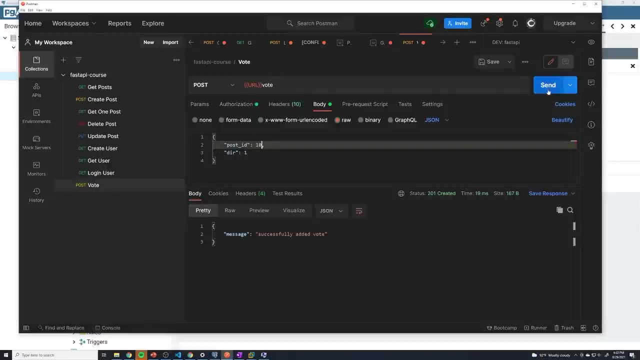 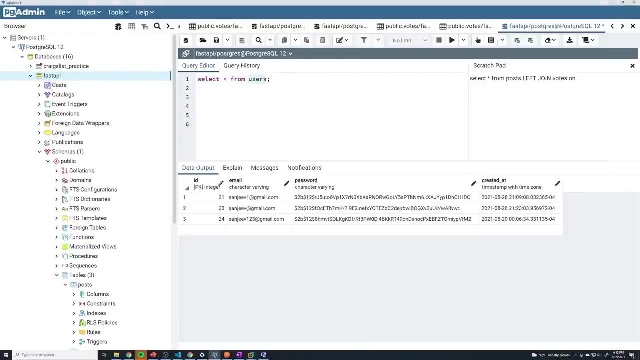 My login. Alright, we've logged in And I'm going to vote on post 10 as well, on this guy, And then we'll grab some random vote, 15.. Okay, and so we should have a decent number of votes now, And I purposely made it so that. 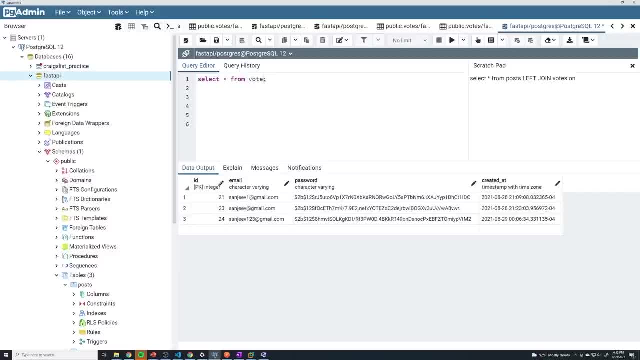 one of the users didn't vote, just so that we can take a look at what complications that add. Alright, so we have all of these votes And we've got the user ID and the post ID, So now let's set up a join. So I'm going to select star from posts And I'm going to 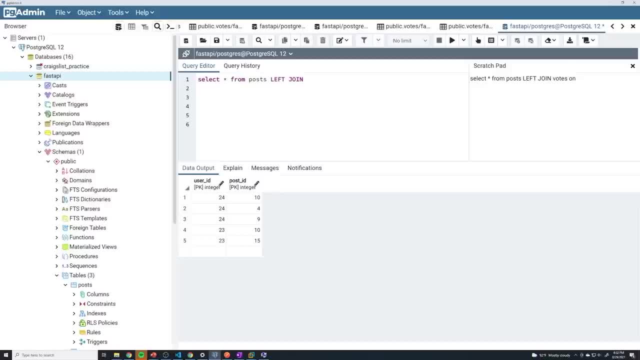 start off with the left join And we'll say we want to join with the votes table And the field that we're going to join on is on the posts. we're gonna grab the dot ID and the and, wherever this is equal to votes- dot, post, underscore ID- we want to join the table. 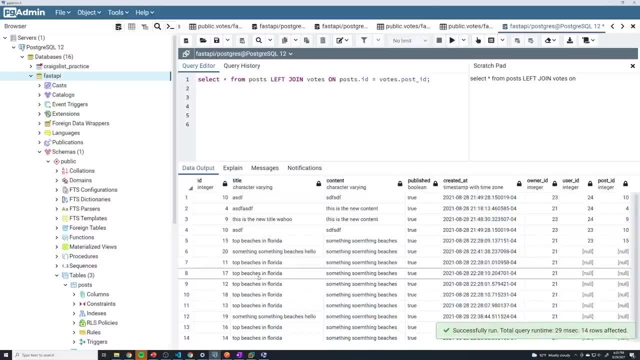 So let's run this And let's see what results we get back. Alright, and so you can see that. hey, look, a post with an ID of 10. It looks like it does have a vote, So this is one. join right here, But then you'll notice that if I go, 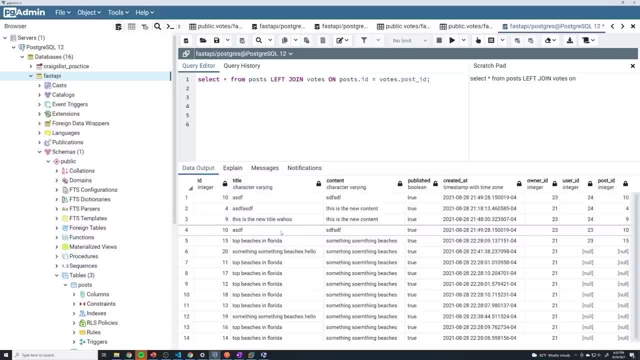 down, you'll see another entry. So this doesn't mean in our database that we have two posts with an ID of 10. is just saying that since we joined them we have to go down the list, see where they match and then print out a row. that's going to print out a row for every. 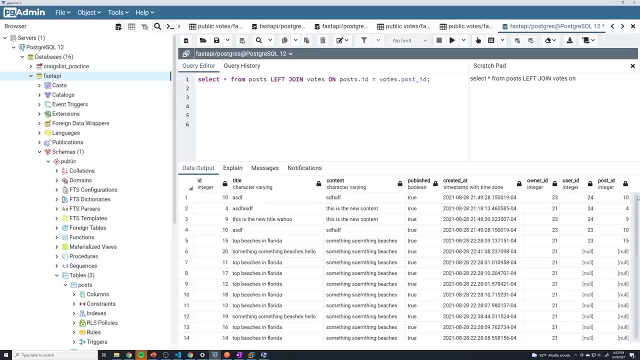 single time. the post ID matches the post underscore ID of the votes table, And so, since we have two votes for the same exact post, that means we're going to get two different entries doesn't mean there's actually two posts in our table. It's just the way that the joints work And I strongly recommend like if this is. 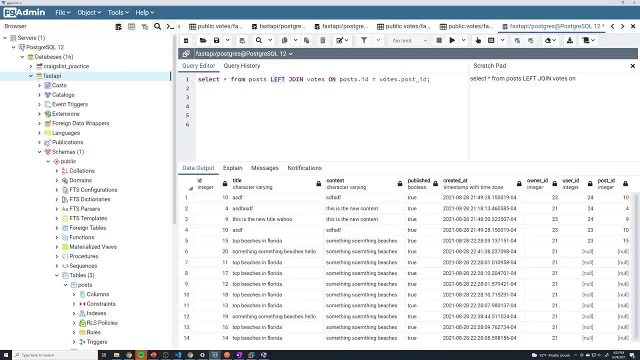 still a little confusing. keep reading that document and play around with it If you want to see the opposite. Actually, before we take a look, let's just take a look at a few other things. You can see we've got post with four And we can see that there's one vote for that, because there's 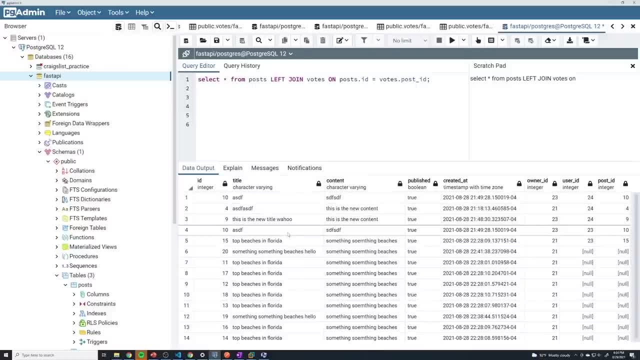 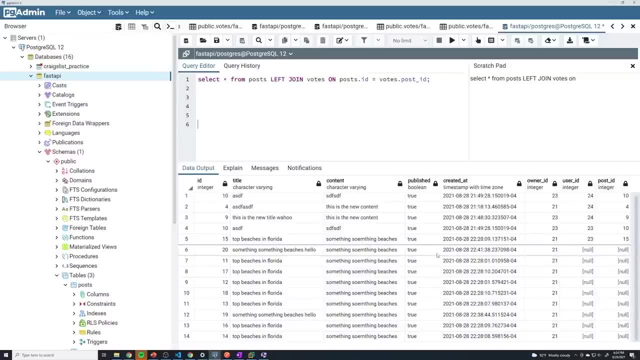 no other entries here with for an ID of four, And then we can see all of these posts that have no votes whatsoever. So that's what the left join gives us, because anytime we have a post which is the left table, since we do a left join, it's going to list those posts And I'll just put. 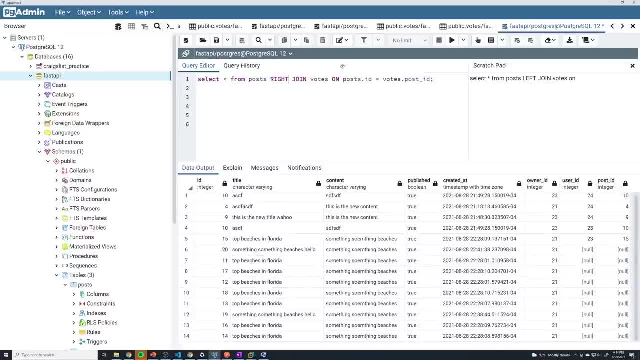 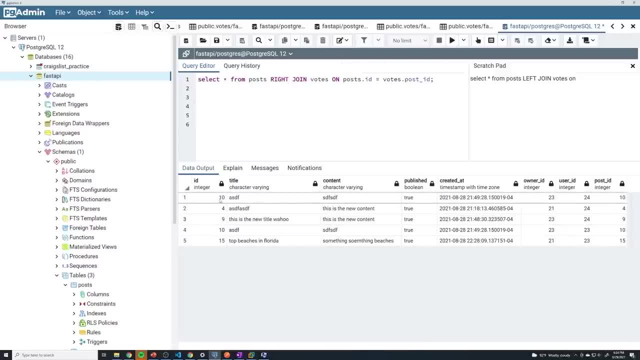 null on the right side, Whereas if we change this to a right join, it's going to do the exact opposite. On with the right join, right once again. it's going to look for any time the the ID here matches the post ID and it's going to spit out a row And then the same thing goes. 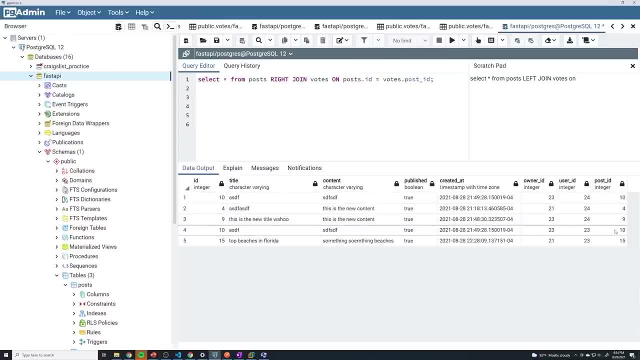 for the post with an ID of four, And then once again, you can see 10 shows up twice because two users voted on it, and then 15 and so on, but then you'll see nothing else, And the reason for that is: we did a right join, So it's going to show us all of the votes and their corresponding. 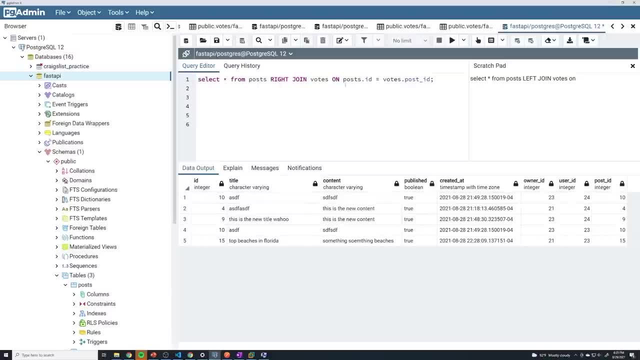 post. However, it's also going to list out any votes because it's a, it's a right join that don't that aren't associated with the post. Now all of our votes have to be associated with the post because we put in that constraint, that check. So that's why we don't see anything with a null on. 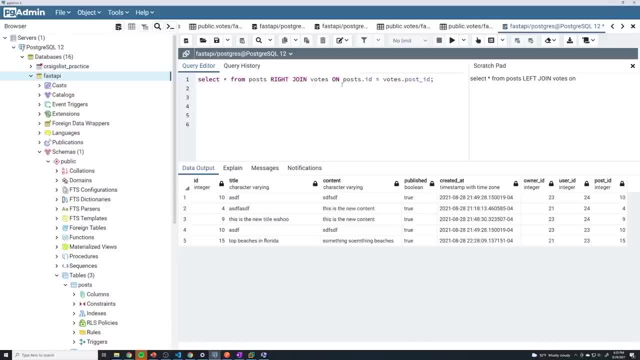 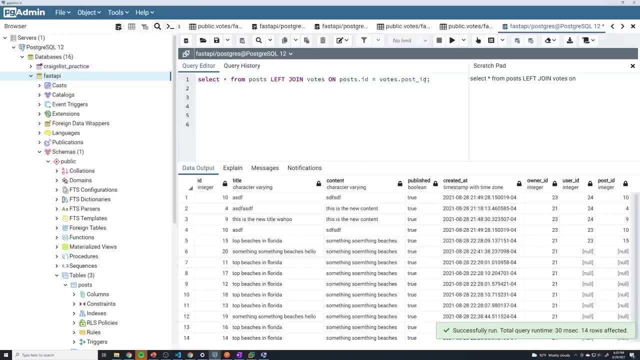 the left side, because that's just the way our tables have been set up, So hopefully that didn't confuse you guys. we're going to change this back to a left join, And what we're going to do now is we're going to do. I want to be able to count the total number of votes for each and every post. 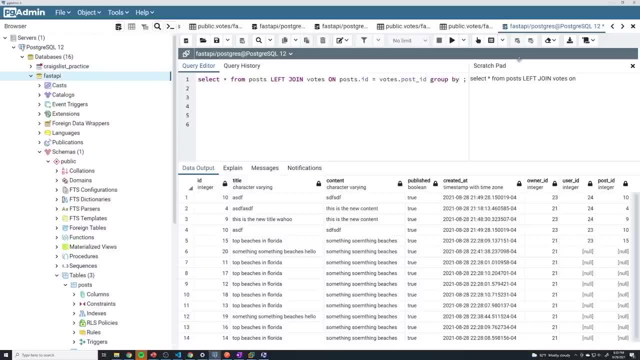 So we're once again going to do the group by. So we're going to group by postid, So we'll group them together and then count them. And for columns I'm just going to say we'll say postid And then we want the count. So we'll start off with the star And let's see what. 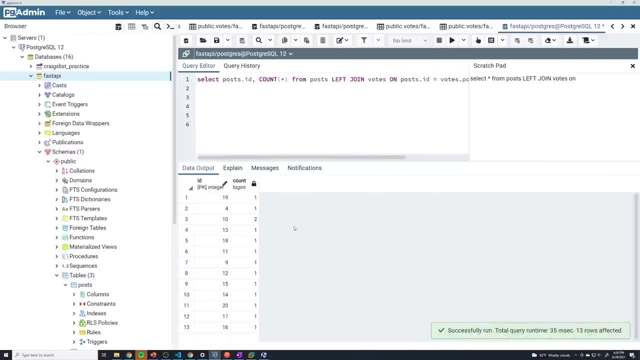 happens. Okay, so we can see that. you know post with an ID of 10, we know it has two votes, But then everything else has a value of one. This is not correct. We know that a whole bunch of posts don't have a value of one, But, like we covered in the previous 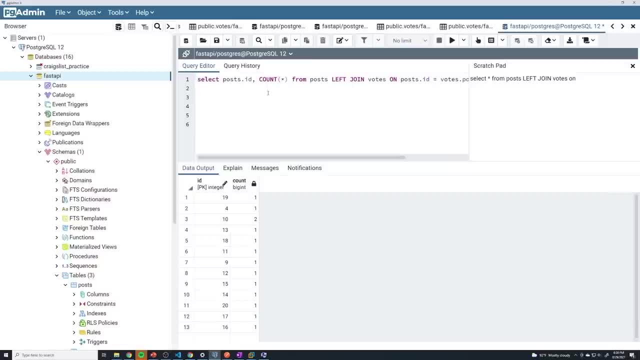 lesson. anytime you have a value of null, then it's going to count that as one. So I'm going to run this- the previous query, remove the group of by, And I'll show you guys exactly what I mean. Now, if I run this- oops, there should be a star. 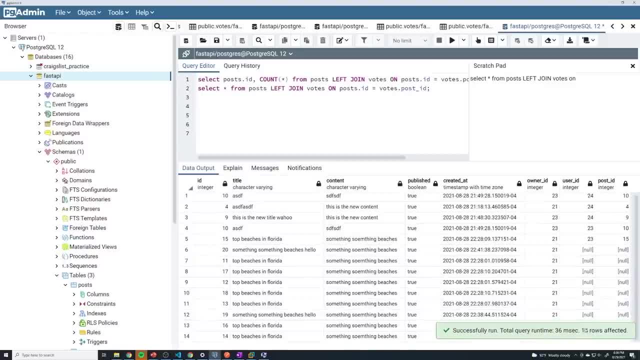 All right, look at all of these posts that have a value of null. It's going to count them all as one in this case, And we don't want that Right. That's why that's what happens when you do star in the count field. So instead, what we're. 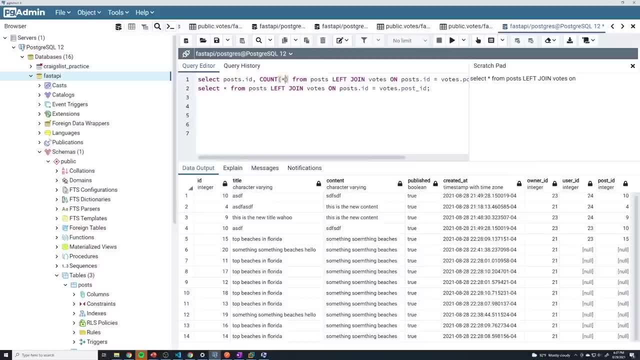 going to do is we're going to provide a specific column to count on, so it doesn't count the null values. So what column should we use? I mean, we can really use any column. I think it makes sense just to do We have to grab one of the columns that are null in this case, So we'll get votes. 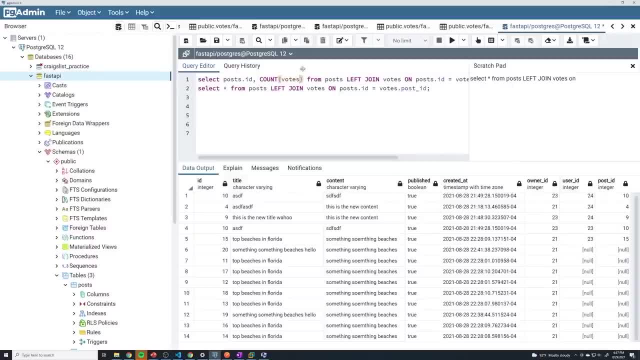 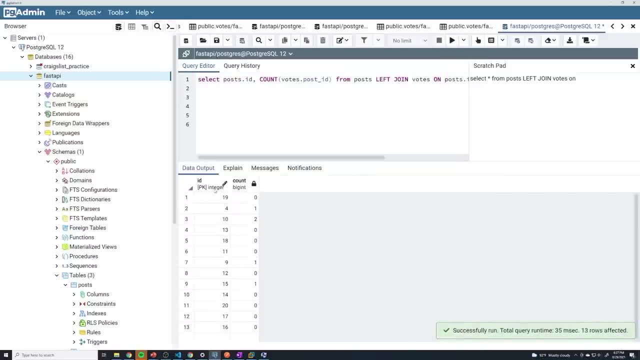 dot. post underscore ID. So now, look at that. we get the post ID And then we get how many votes they have all together, or how many likes, And instead of just grabbing the ID, I'm going to actually grab everything from the post table. we can run that And this is the exact. 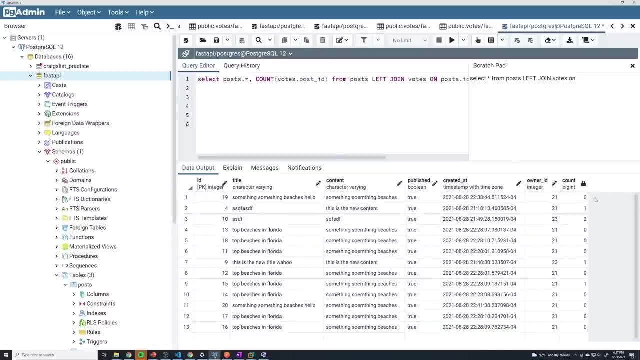 query that we're looking for. we get the post information and we get the number of votes And we can rename this Because I don't like calling account. we can rename it as you know. votes or likes doesn't really matter. 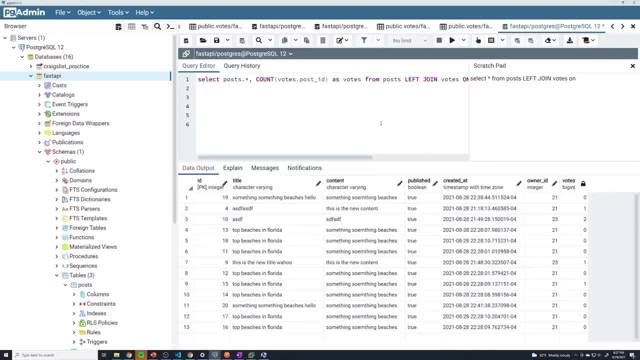 And there you go, guys. And if you guys want to query for an individual post and get the total number of votes, it's actually very simple. It's the same exact query. we're just going to provide a where condition, And so here I can just say: where post ID equals one, Well, actually I 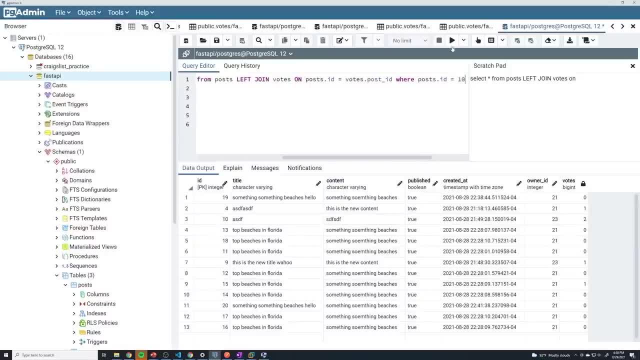 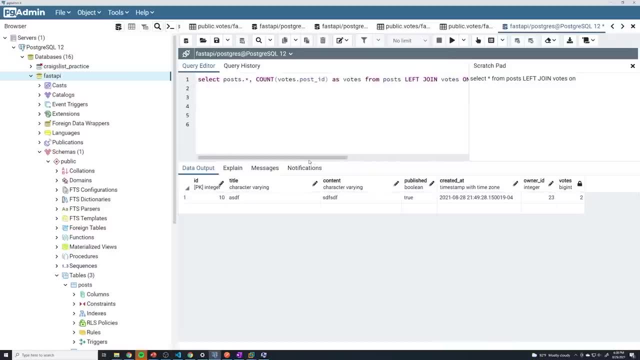 don't have a post ID of one, so I'll grab a post ID of 10.. And so now I get my one post And we can see that he should have two votes, Alright, and so that's how we do this with. 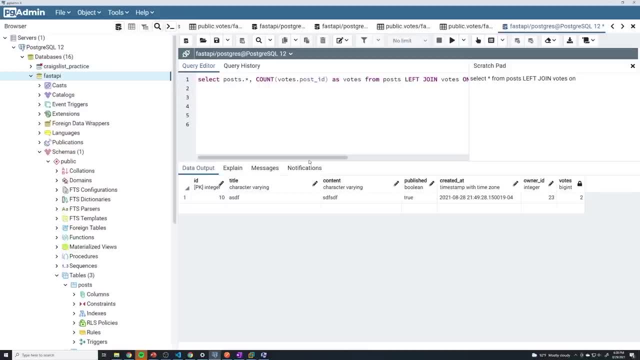 raw SQL. Hopefully this wasn't too complicated. Like I said, I strongly recommend you spend a little bit of time going over joins and practicing it with your own tables. Don't just use posts and votes If you can probably come up with simpler tables to work on this and understand it a little. 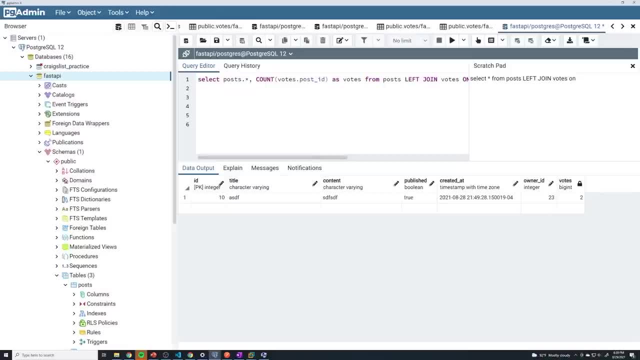 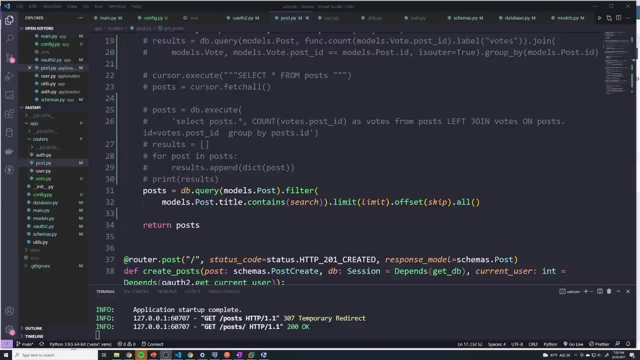 bit better, But I think that's going to wrap up this video, And so go ahead and just save these queries for now, so that we can reference them later. In the last video, we saw how we can gather information from two different tables by making use of joins, And so we saw how to do that with 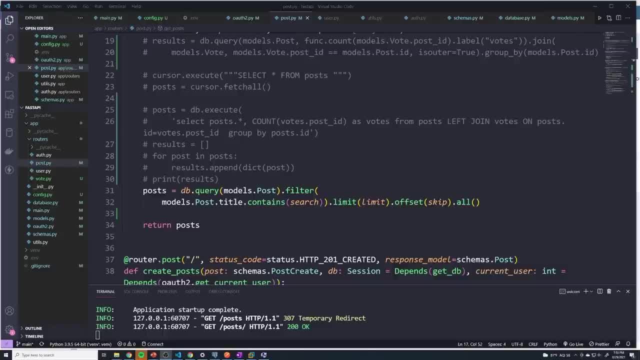 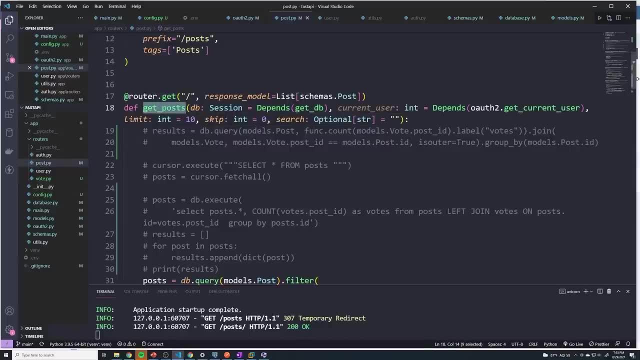 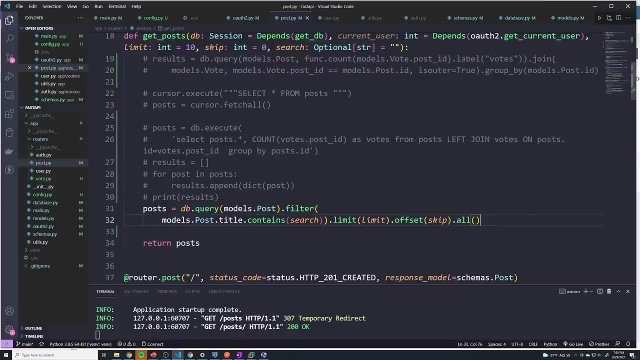 raw SQL. And now we're going to see how we can perform joins using SQL alchemy. And if you go to your post router, we're going to go to the get posts path operation, And so we're going to kind of just take this step by step and see how we can slowly build out this query so that we can 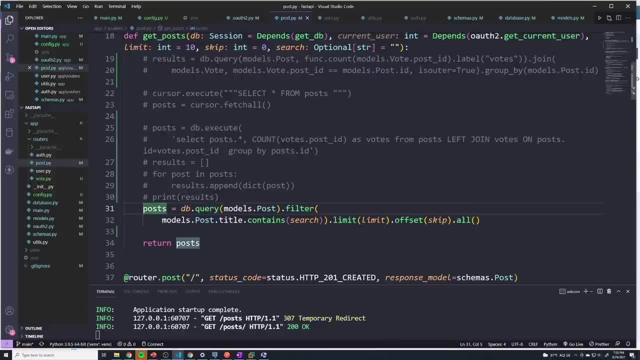 actually perform a join. If you take a look at the current query, what we can do is just ignore all of the filter stuff first, And so really the the meat of this query is just db dot query And then you pass the model. 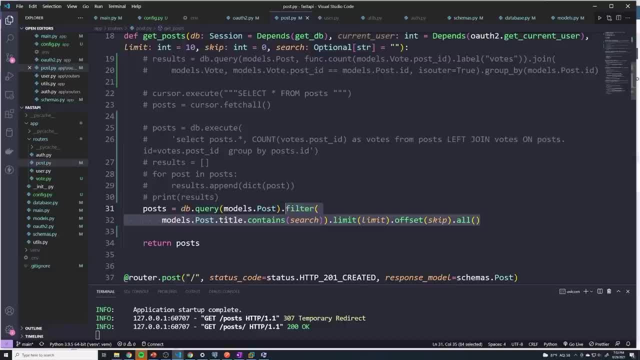 And that's going to get every single post that we have in this table, And then we perform all of these filters to kind of drill down. So we're going to start off with the same thing And I'm going to save this new query as results. Or or we could just say posts underscore votes maybe. 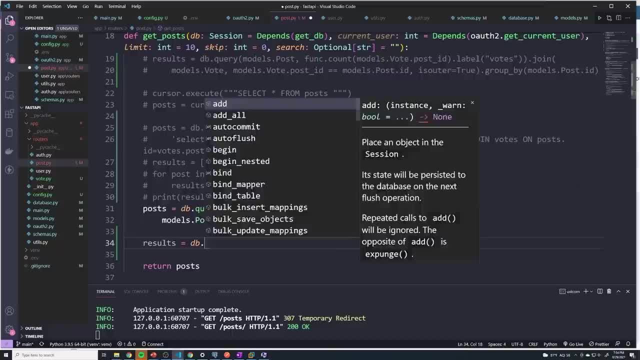 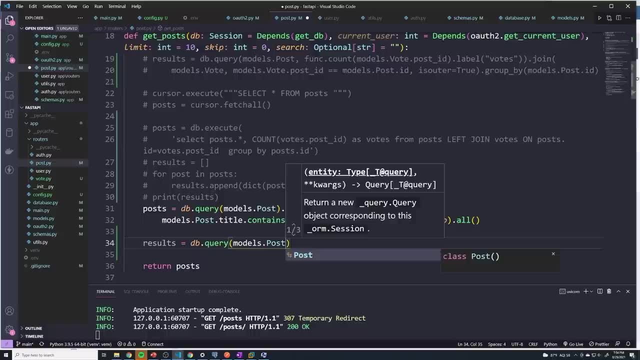 and we'll just save it as results. And so we're gonna start off with the same exact query. we'll query models, dot post And we're perform dot all, actually remove the dot all. And the reason I don't want to do the dot all is I don't actually want to query the table, I just want to actually 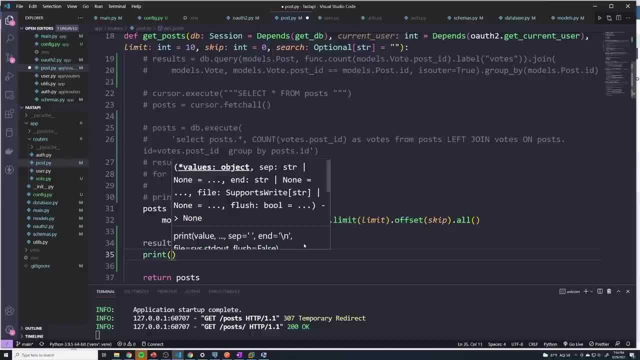 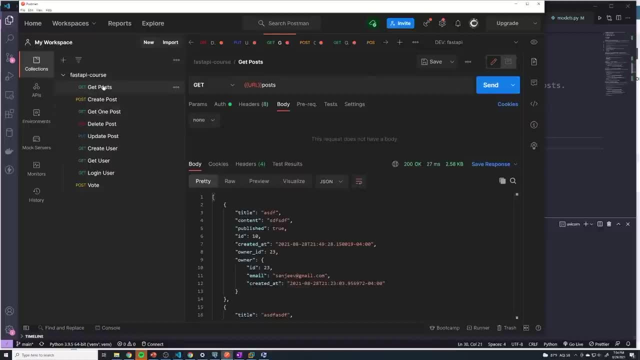 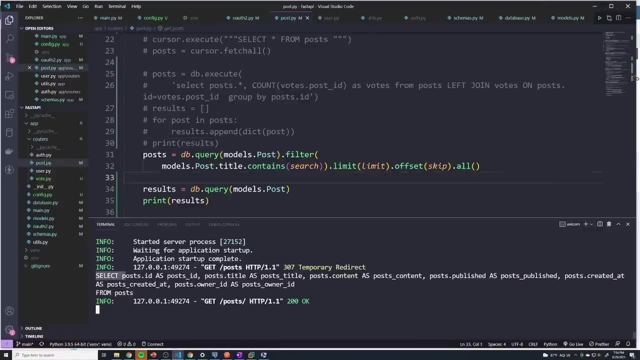 see the raw SQL that's generating And now we can do a print results. I'm going to bring this up a bit And we're going to just send a query to the get all posts And you can see the raw, the SQL that it generated. So it's going to select and then basically select every column and then 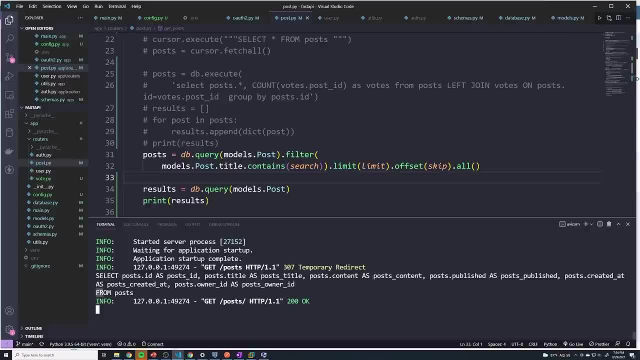 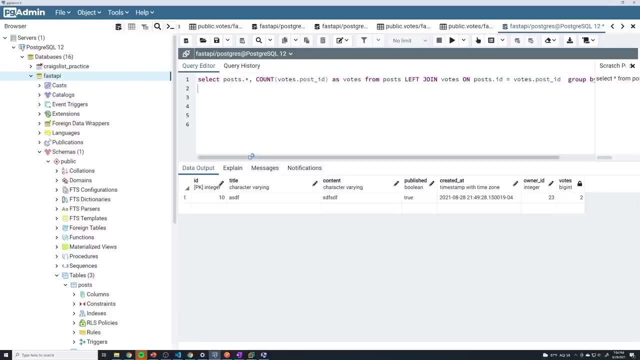 rename it accordingly And it's just going to get that from the post table. So it's getting every single post, That's all. So everything is pretty straightforward at this point. And if we go back to our PG admin, let's actually take a look. Let's take a look at what our SQL query actually looks. 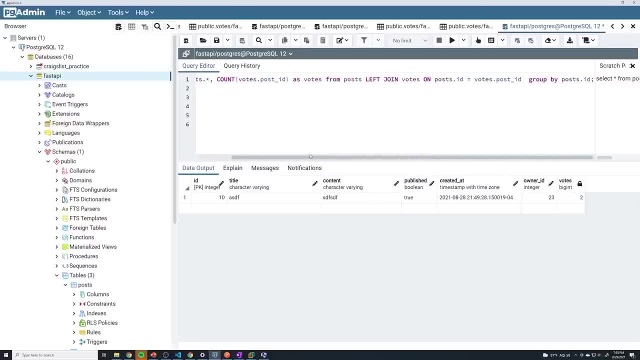 like, And so you can see here there's a whole bunch of things going on. But the next thing I want to do is I want to actually start to perform the join. So I want to join on the votes table. So let's take a look at how we can do that. 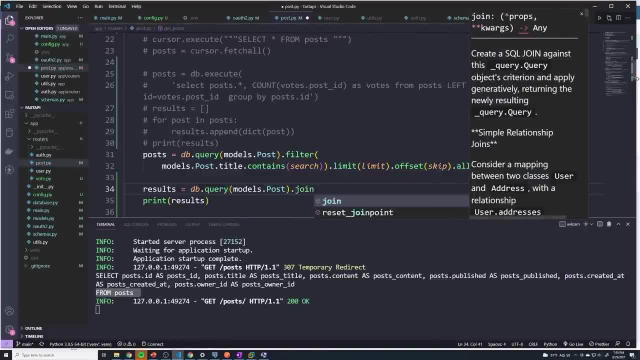 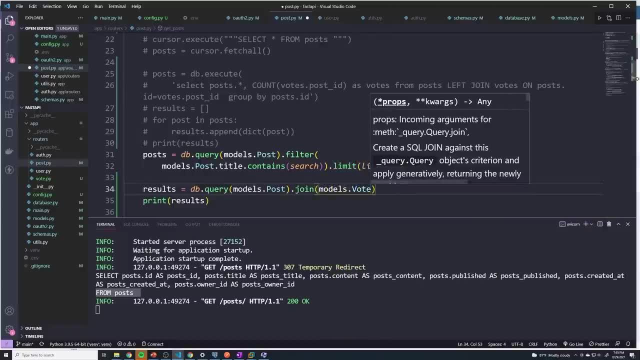 And to perform a join with SQL alchemy, I can just say join, And then we have to specify the table we want to join. So this is going to be the models dot vote. And then the second thing is: what is going to be our the, what is going to be the column that? 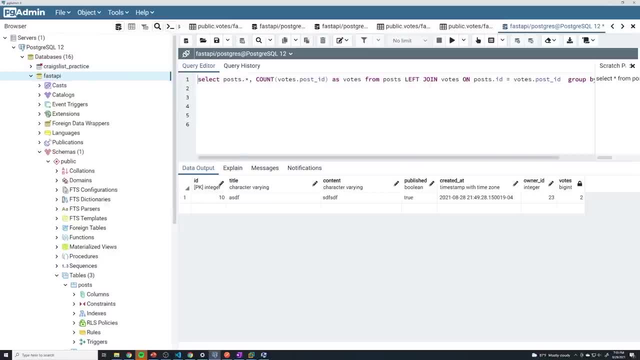 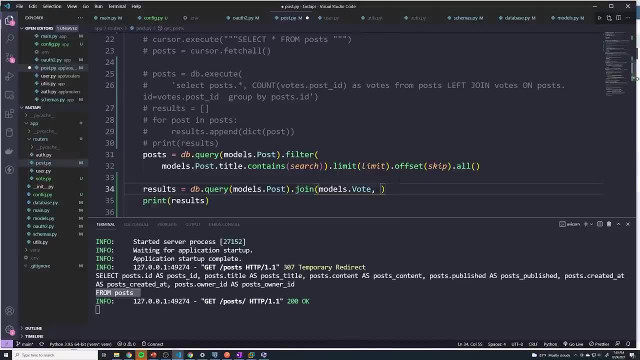 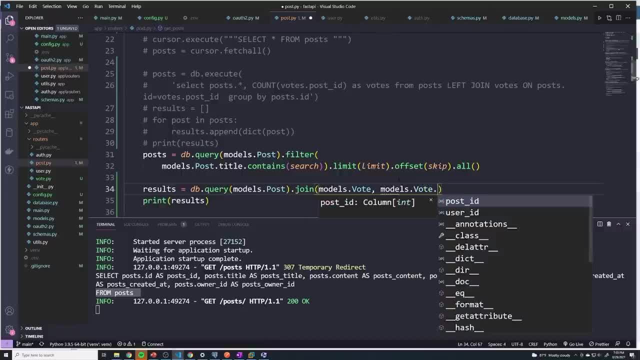 going to do the same thing here. I'm going to say models dot vote dot post underscore ID equals, equals. and then we'll say models dot post dot ID. whenever they're equal, we're going to join the table. Now, the thing about this join is by default with SQL alchemy. 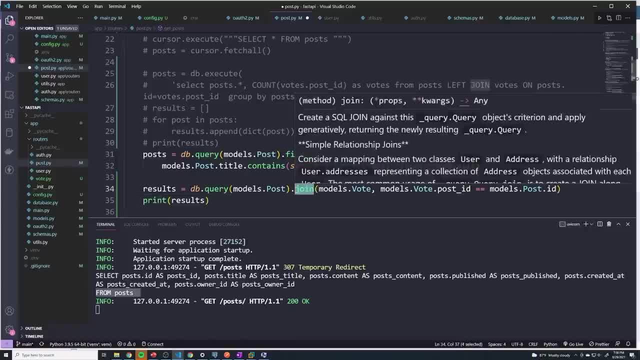 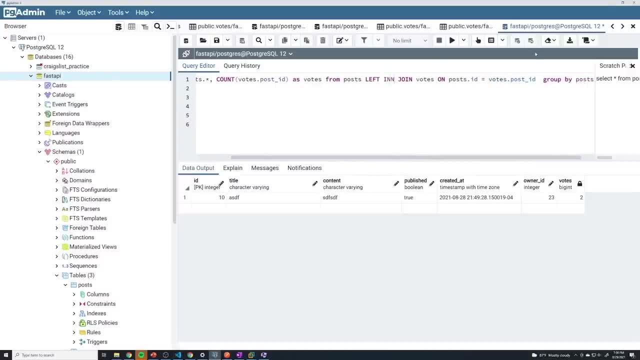 this is going to be a left inner join And the word inner is going to be a little bit new for you, And it's because there's two different types of left joins: you've got left inner and you have left outer, And I don't want to spend too much time kind of diving into what's the 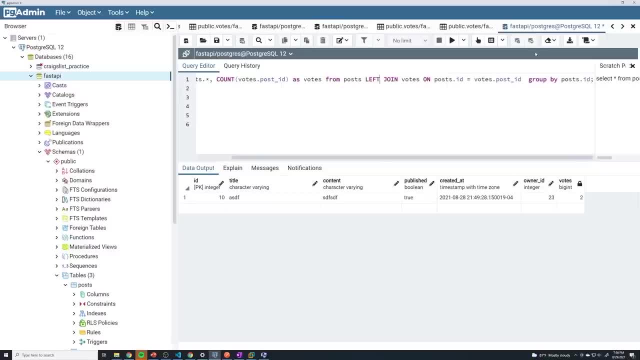 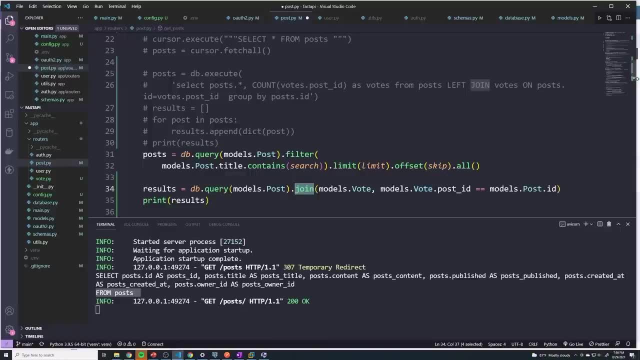 difference. just know that if you ignore the keyword, it's going to by default be an outer. So what we want is an outer join. However, SQL alchemy by default uses inner joins. So to actually set this as an outer join, we have to pass one more thing. 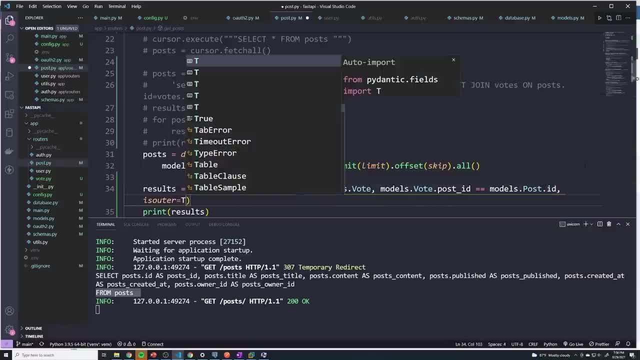 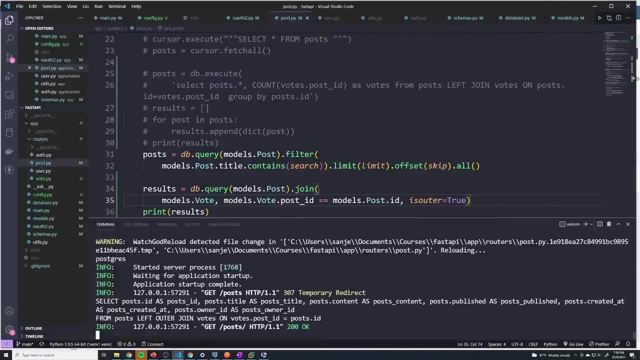 which is going to be is outer equals true. So this is going to make this a outer, left outer join. So we've got our join at this point And what I'm going to do now is save this again And let's take a look at our query. I'll send something And now we'll take a look at our query. we can. 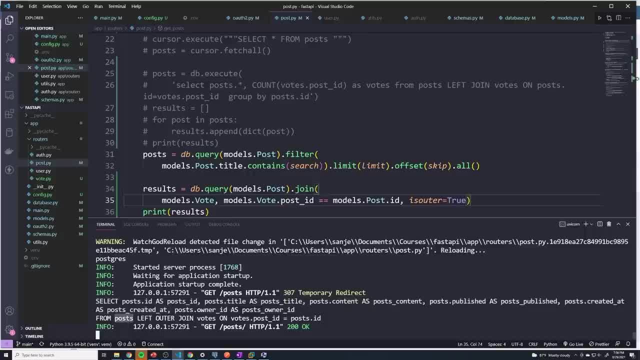 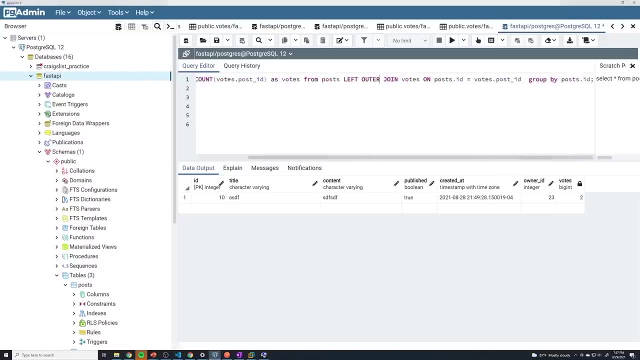 see that, okay, we're going to select everything from our post table. then we're going to perform a left outer join with votes on the table votes whenever votes that post ID equals post dot ID. So we're almost there. The next thing that we have to do is we have to group by post that ID. 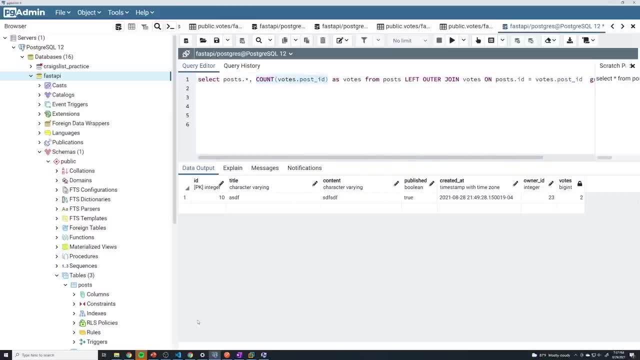 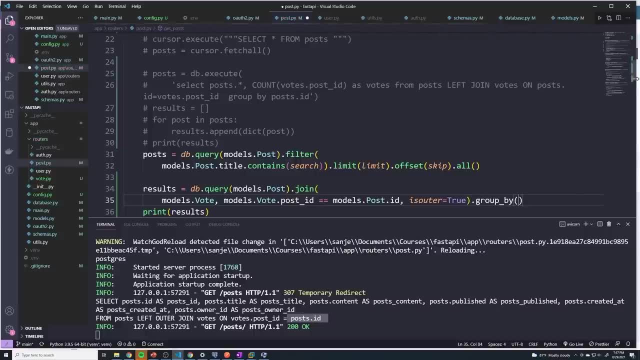 And then we have to perform the count on votes. that post underscore ID And so if you can take a guess, this has to do group by. we can just do dot group underscore by and then we specify the specific column. So we'll do models dot post. 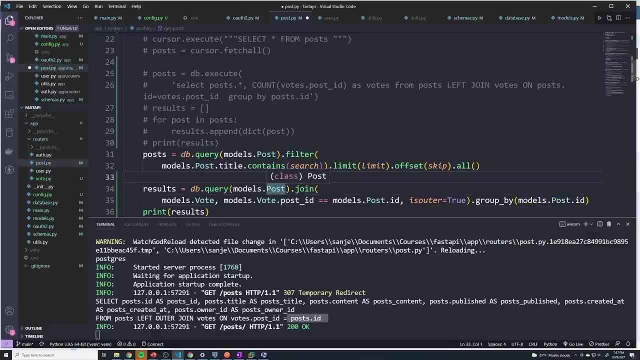 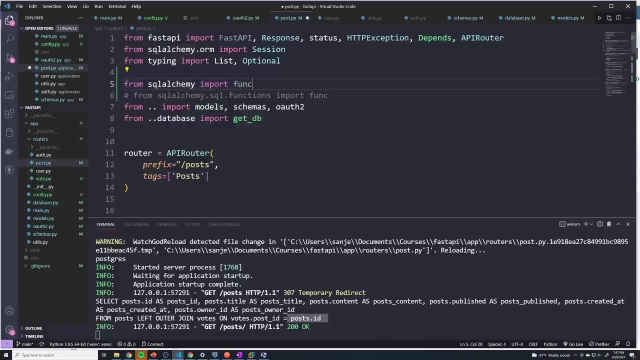 dot ID, And then we have to get the count. So we'll go here And I'm going to say: well, first of all we have to import a function. So what you're going to do is, from SQL, alchemy, import funk, And so this is going to give us access to functions like count. 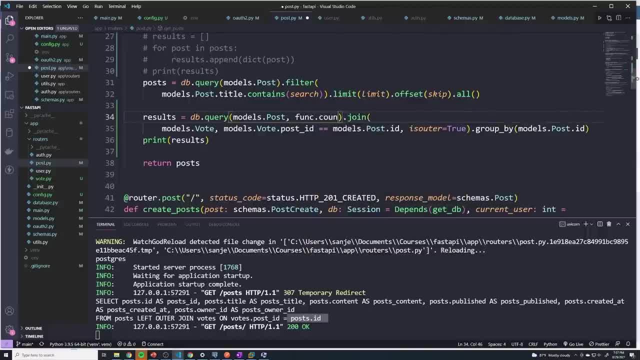 I'm going to say funk dot count. And then we'll say models dot vote dot post underscore ID. We'll save this And I'm going to send this and let's take a look at the query once again. And so we've got select posts, all of the post columns. good, good, good, good. 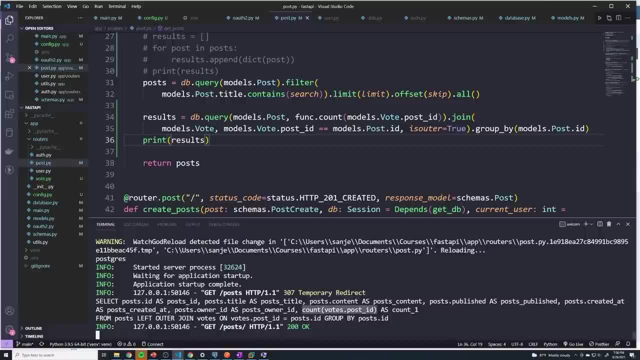 And then we get to count Right and it's going to perform the count. That's all right. However, we're naming it As count one. I don't like that. I want to name this something that I will understand, So maybe. 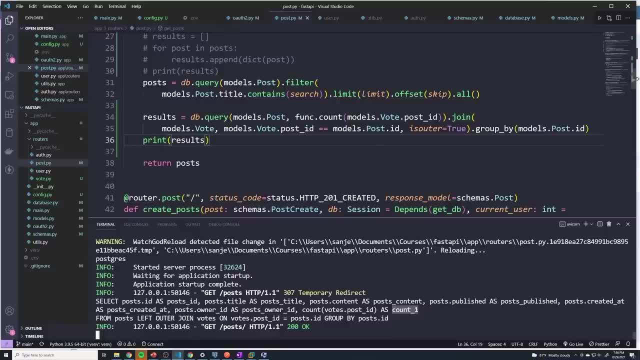 something like votes. So we have to figure out a way to rename this column, And if you want to rename this column, you just say dot, label and then the name that you want to give that column. So we're going to call this votes, And so let's test this out one last time, And now we can see. 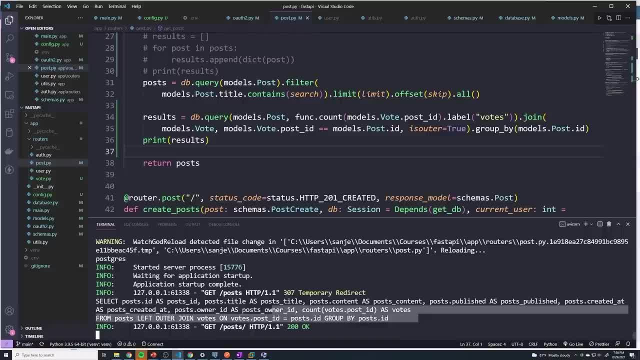 that the column is called votes. So this is exactly what we want. This is the exact query that we generated In PG admin manually. we're just doing it through SQL alchemy And what we're going to do is, well, let's actually perform the query. We'll do, dot all. 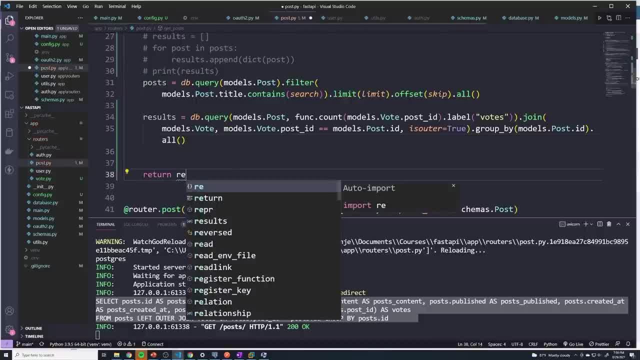 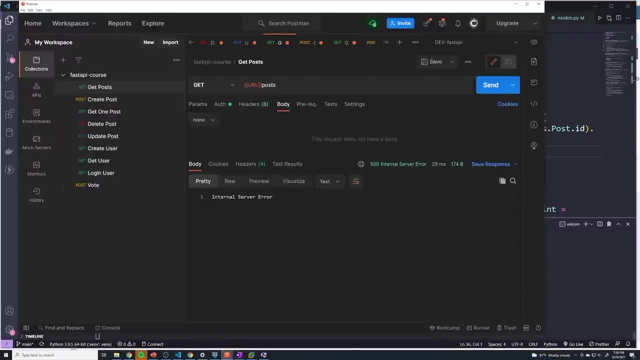 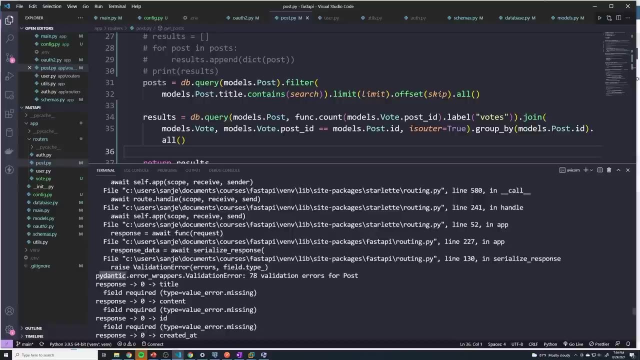 don't need the print anymore And we're going to actually return results And let's see what happens. So now, if I send a query, it's giving me a whole bunch of errors, And if we scroll to the top of the errors we can see that these are all pydantic validations. 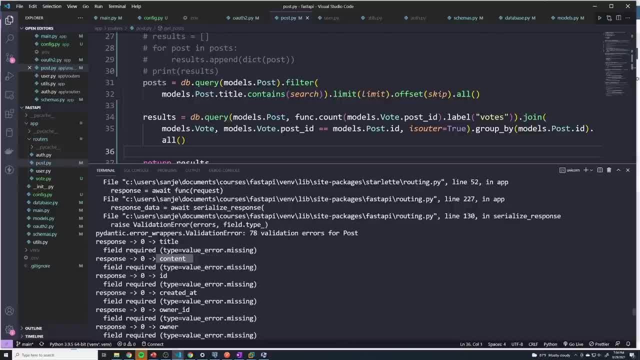 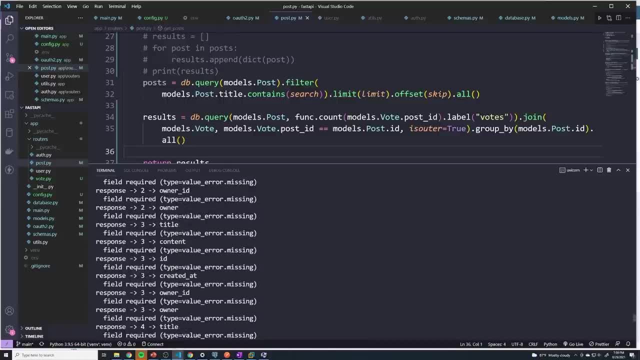 And so it's saying that, hey, there's no title, there's no content, there's no ID, there's no owner ID, there's no owner. all of these fields seem to be missing. And why exactly is that? Well, let's take a look at the response model. So the validation. 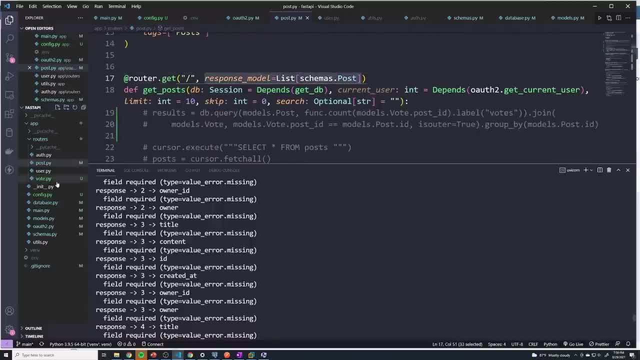 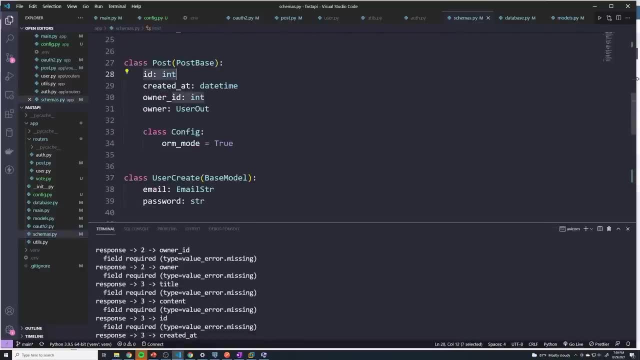 is happening because we use this response model of schemas- dot, post- And so if we go to schemas and we find our post object or post class, you can see that expects an ID created at an owner ID, an owner and all of that good stuff And it's. 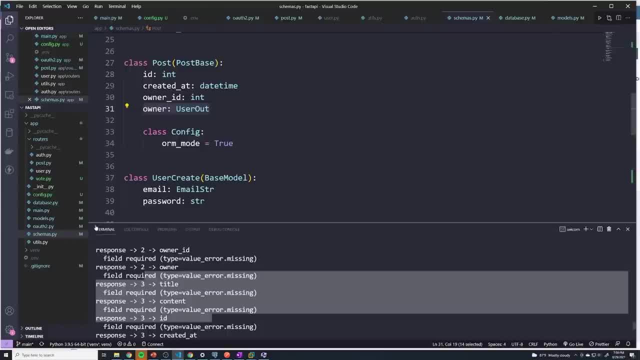 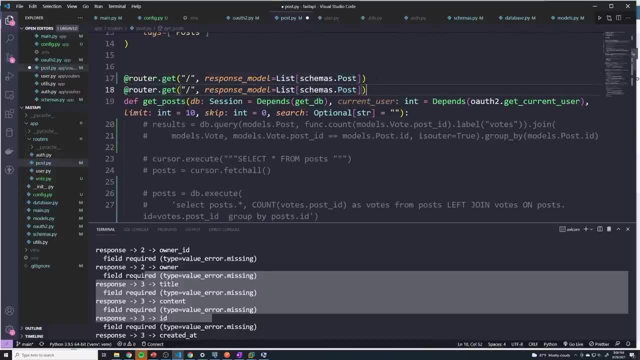 saying that none of these have been set, So it looks like there's something wrong with our query. But just to make this a little bit simpler, what I'm going to do is I'm actually going to remove the response model. So I'm going to just comment out that: remove the response models. 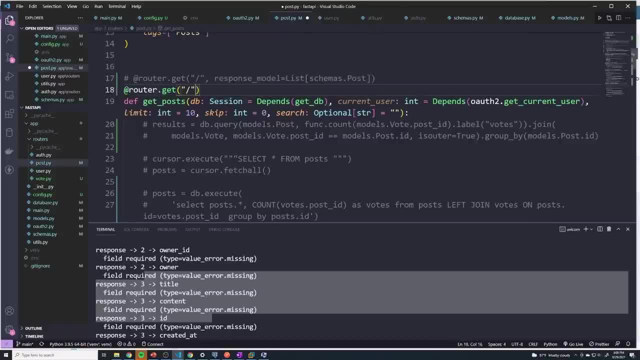 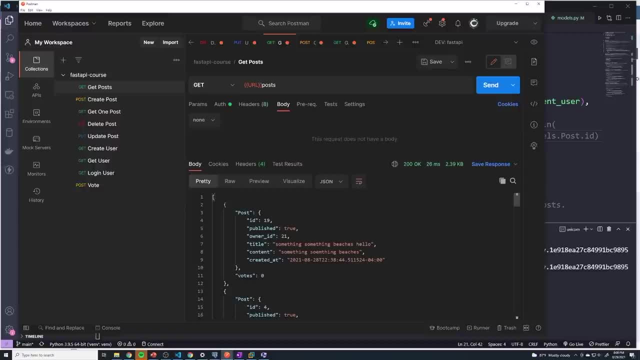 we're not actually performing any validation And we're gonna see what this looks like now. So when we retrieve the data, I want you to take a look at what this looks like. So this right here is one specific post, And so after our changes, we can see that we've got a property called post and then within there we 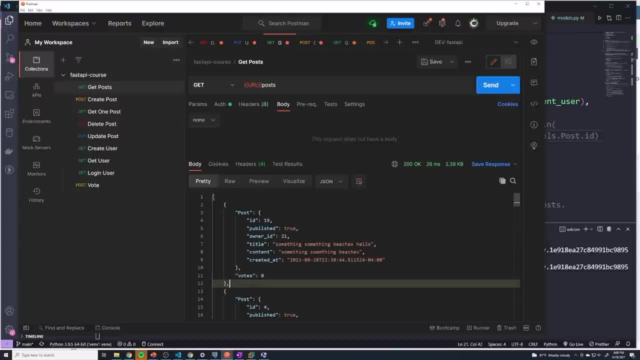 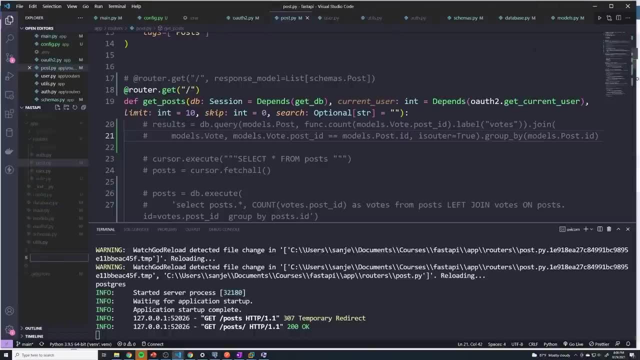 have id published and so on, and then we've got a property of votes and i'm actually going to copy this as an example. i'm just going to create a new file and i'm just going to say we'll just call this examplepy. that's fine, it doesn't really matter. we'll delete this in a bit. so this is. 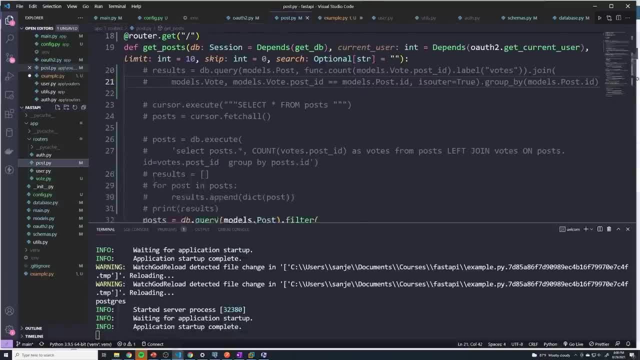 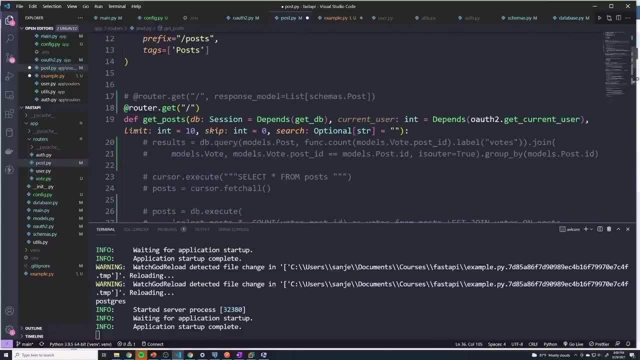 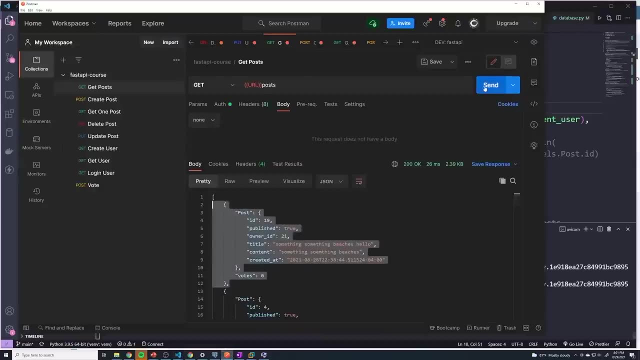 what it looks like and when we go back to our path operation, i'm going to return posts and we can actually return the response model just to see what that looks like. and so now if i do a query i need to save and if you take a look at the query, this is what it looks like in a working state before we set up. 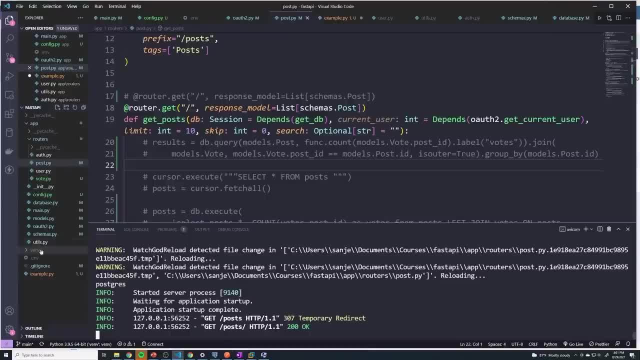 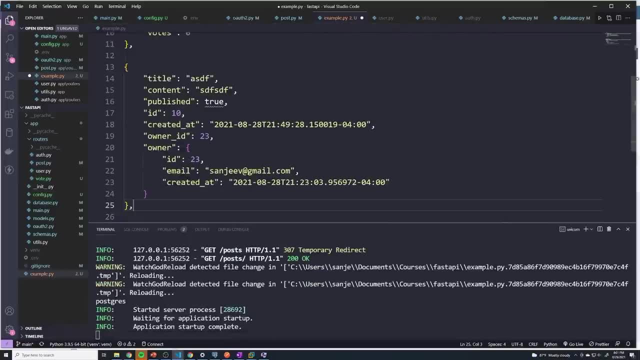 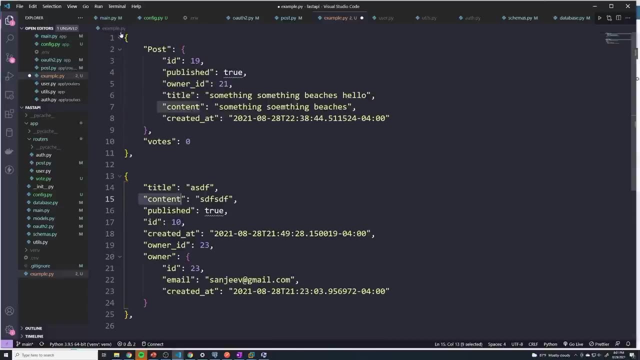 the joins. and if i go down to my example, where's my example py file? and i'm going to go to my example and i'm going to go to my example and i'm going to go to my. so this is what pydantic expects: expects to get an object with a field of title, content, published id and so on. however, after i 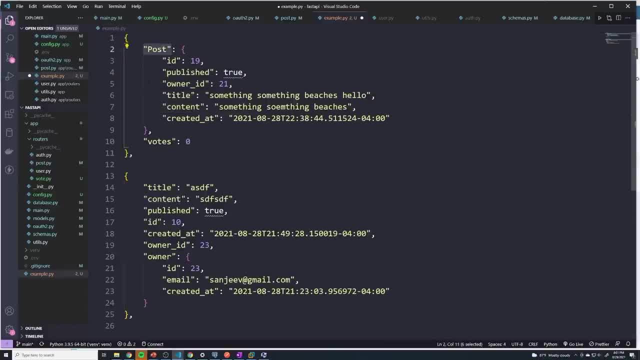 join. something odd happens. we have a field called post and that breaks everything, because it doesn't expect the id and the published and the owner to be under this- uh, this essentially this dictionary right here, and that's why it's throwing all of these errors. so how exactly do we fix this? well, 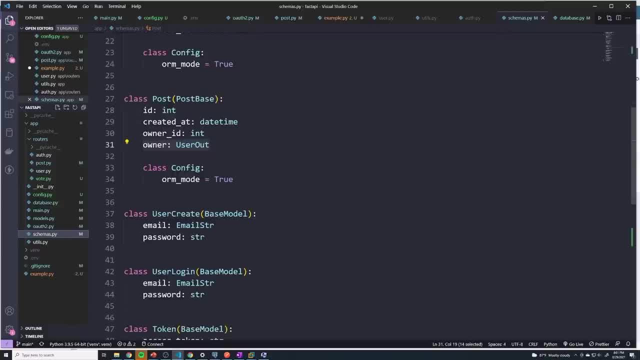 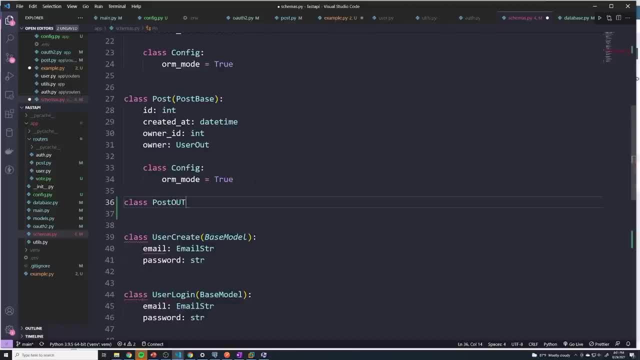 maybe post vote, or i'm just going to call this post out and it's going to be a post base. it's going to extend post base and what we're going to do is we're just going to try to match this as close as possible. so this is going to represent a post object and then we're 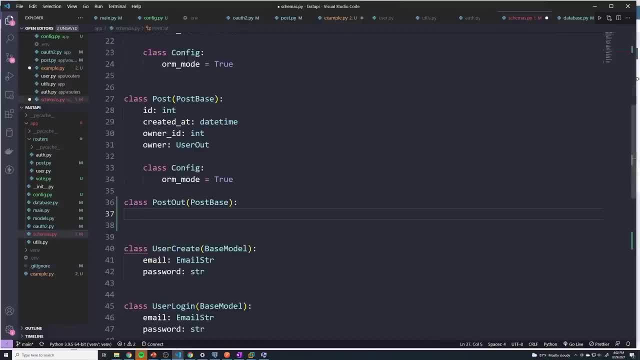 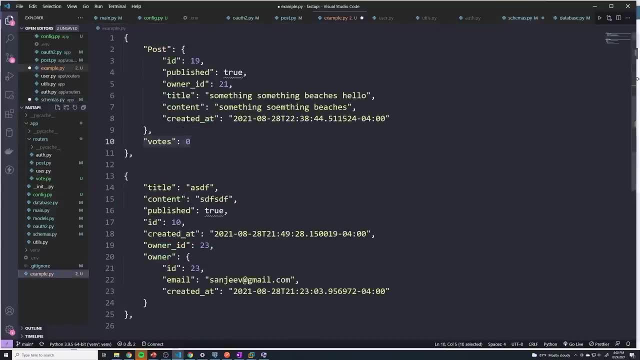 going to have a field called votes, which is going to be an integer. so here i can just say: we have something called post, and don't forget to capitalize it, because our query for some reason returns it with the capital p. took me a little while to figure that out. i was running into a few 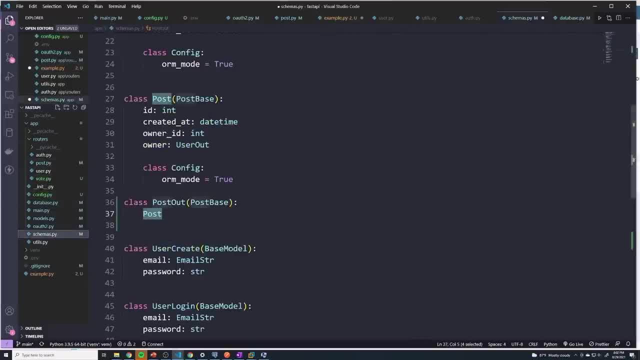 issues. but we can go here and we can say: i want to return, i want this to be of type, and then we'll reference this post right. so all of these fields will be under a field named post, and then we expect something called votes, which is going to be set to an integer. so let's try this out and we'll go. 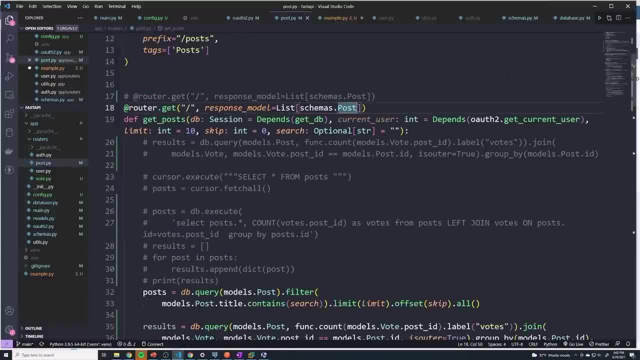 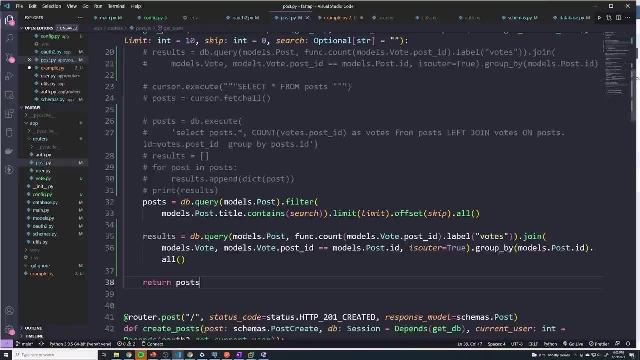 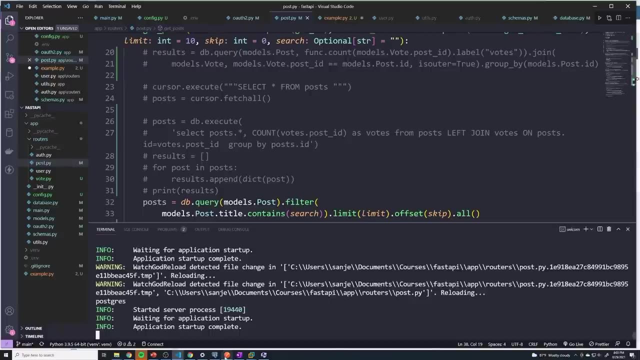 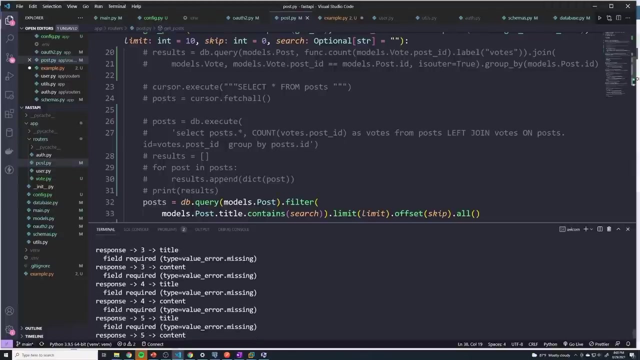 back to our postpy and i'm going to call, i'm going to reference, post out and we're going to return results again and let's just make sure there's no errors. it looks like it's good and let's see what happens now. all right, we got a little bit of an issue and it looks like there's a title, content, title. 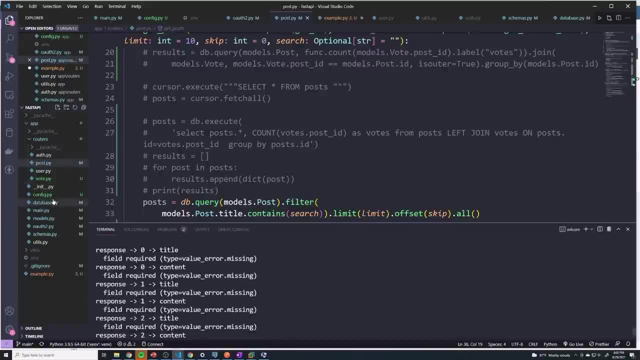 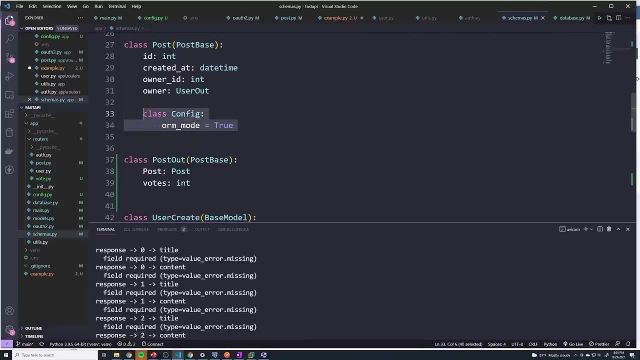 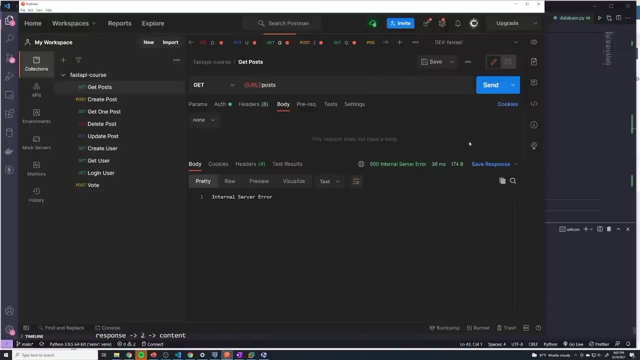 content, a whole bunch of errors, and so the title and the content are missing for both. so what did we do wrong here? this should have fixed our issue. well, let's try adding this class config orm. i think that might actually be what's causing this problem. and now let's try this. 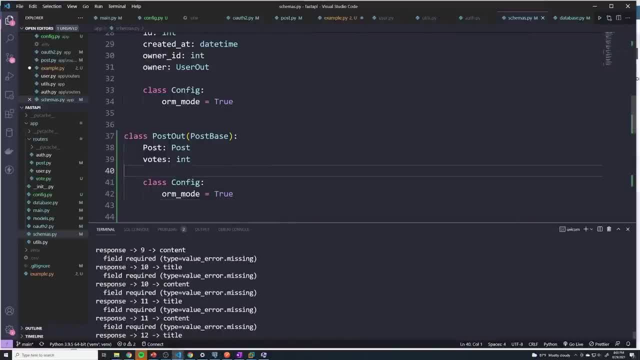 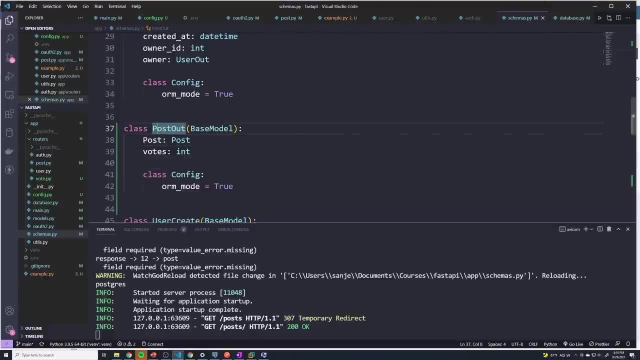 oh, that didn't look like it fixed it. all right, guys. so i was playing around with it and then i don't know what exactly fixed it, but all i did was i had changed this to a lowercase p, and this led to you know us seeing this. 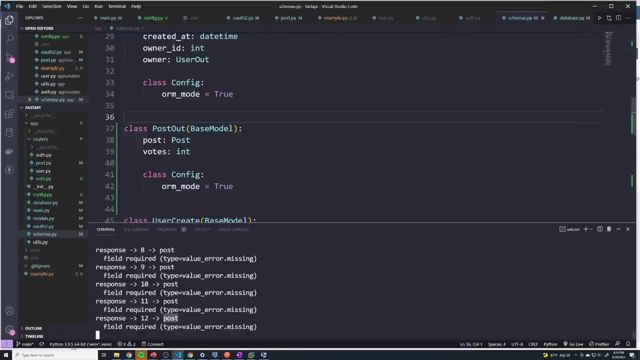 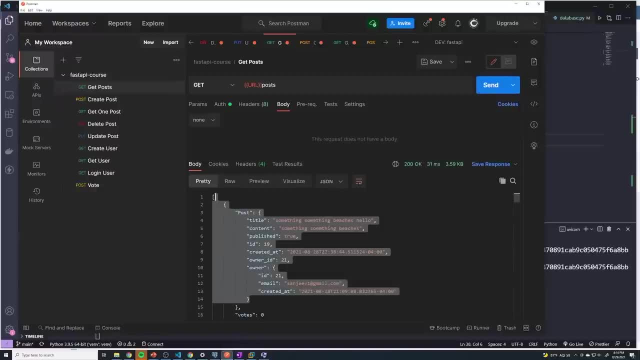 space. and then i was like, oh my god, this is a problem. and i'm like, oh my god, this is a problem, specific issue where it says: you know, hey, this post doesn't exist. and then, as soon as i recapitalized it, all of a sudden it started to to work again. it starts to work now. so i'm not. 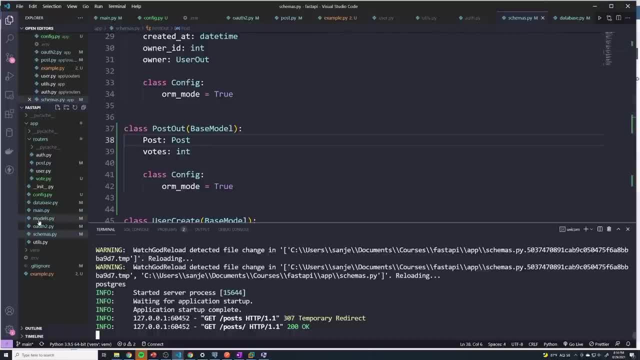 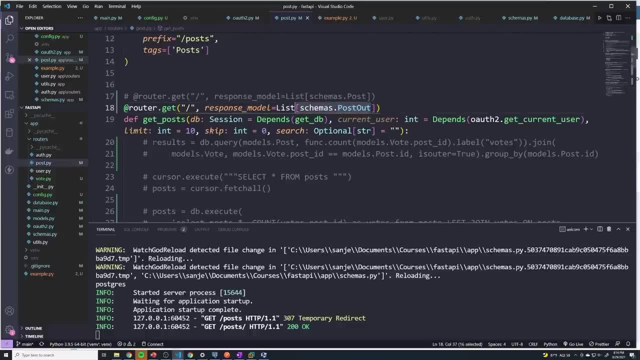 really sure why it broke in the first place. i didn't change any other code. uh, just looking back at my path operation, you can see that i'm now changing my response model to be schemaspost out, and then we're performing the same results query and then returning it for some reason, or? 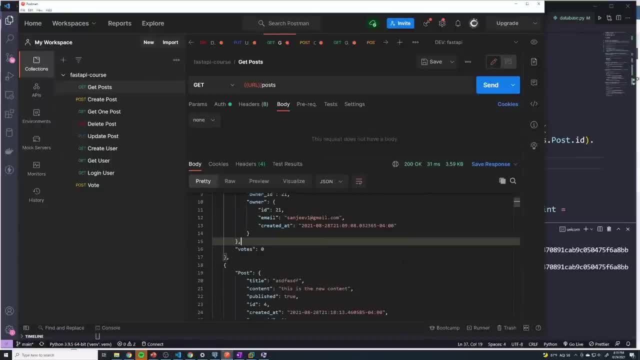 another. it's now properly working. i have no idea what's going on here, so i'm going to go ahead and run it and see if i can fix it. i have no idea what changed. i have no idea exactly what changed, but it's working now. so hopefully you guys don't run into any issues and hopefully 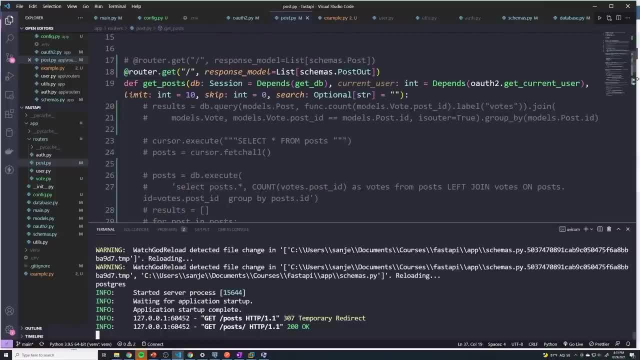 it was just some kind of issue on my machine, but if you do run into the same issue, just try moving it to a lowercase, try restarting the application, then changing it back. i have no idea why that would fix it, but seems to have done something, and so now our results are perfect. we get the 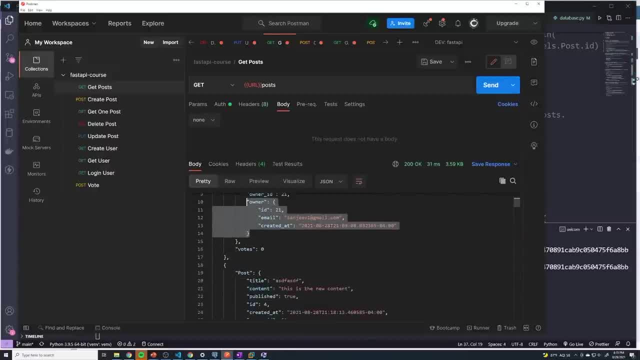 post information. we still fetch the owner, which is fantastic- and then we have the votes and then just double check to make sure that all of your votes are all okay, and so it looks like they all look good. i know that one had two and then the rest. 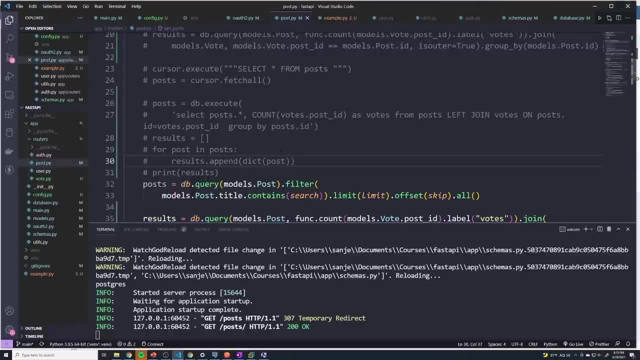 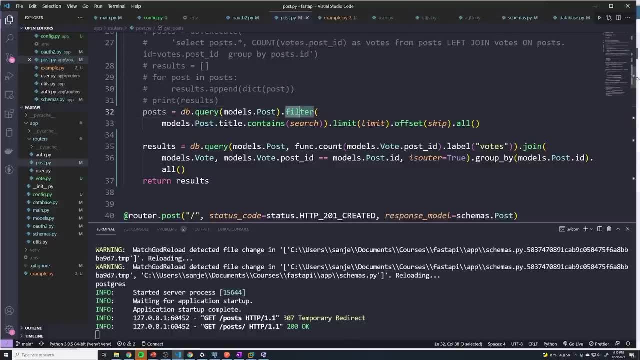 should all have zero. so everything's looking pretty, pretty good. the next thing that we need to do is actually go ahead and add our filters back in, so let's see if i can still filter on all of these, and so i'm just going to copy this and then, before i perform the dot, all i'm going. 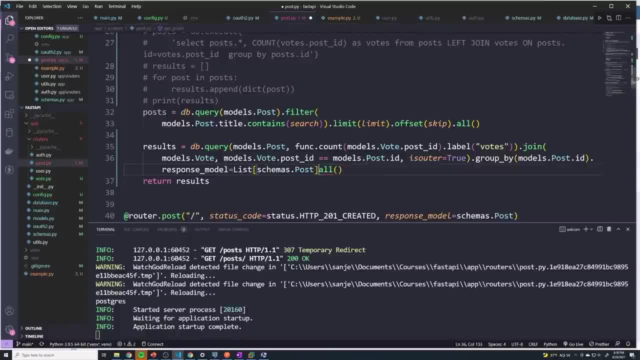 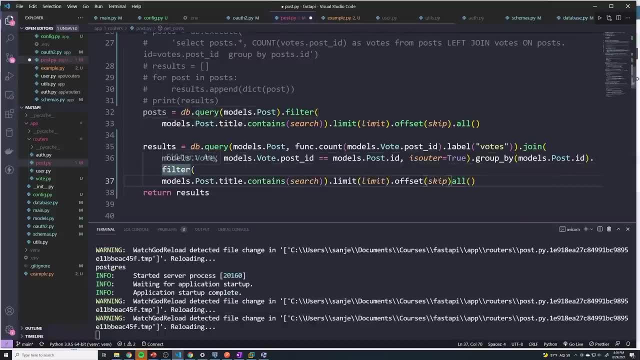 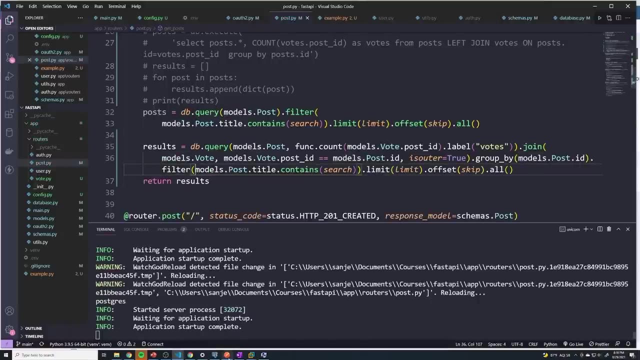 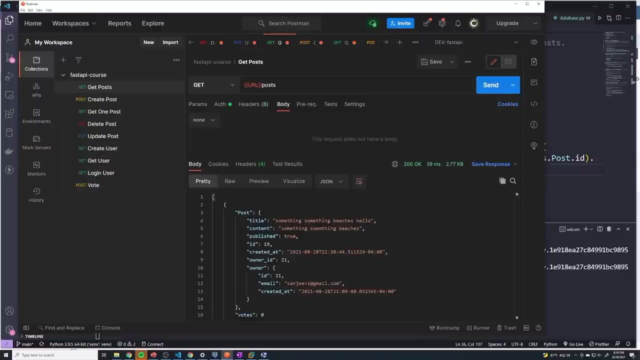 to paste that in there. whoops, i forgot to. i forgot to copy. all right, and then let's test this out again. all right, things are still working, but let's just add a few extra query parameters. so i'll say: search equals beaches, all right, and then 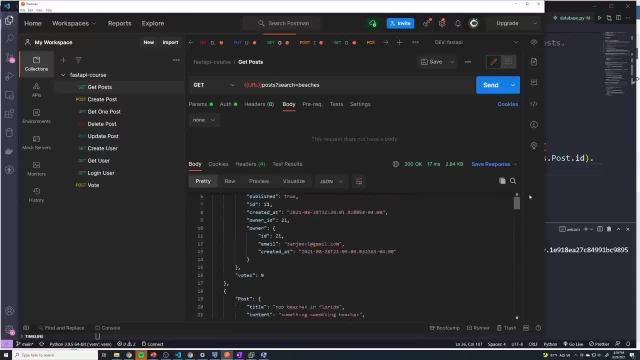 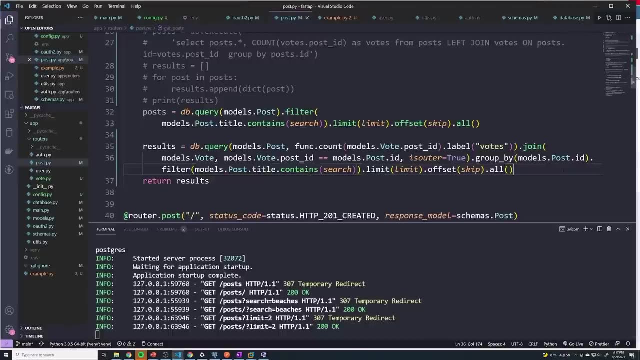 it looks like it should only return posts with the word beaches, and then let's try: limit equals two. remove this search for now. and that works too. so it looks like we get to keep all of the same functionality that we had before, so i'm going to just write this as posts. we're going to comment this out, just for reference. 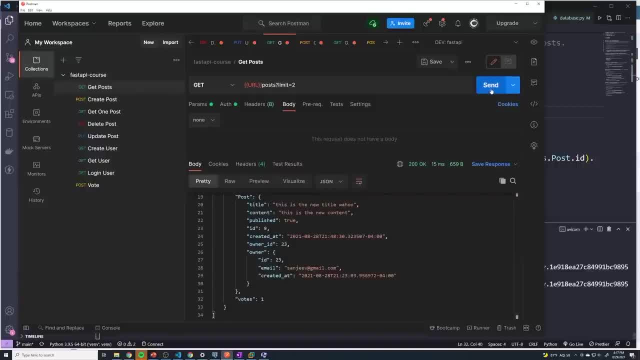 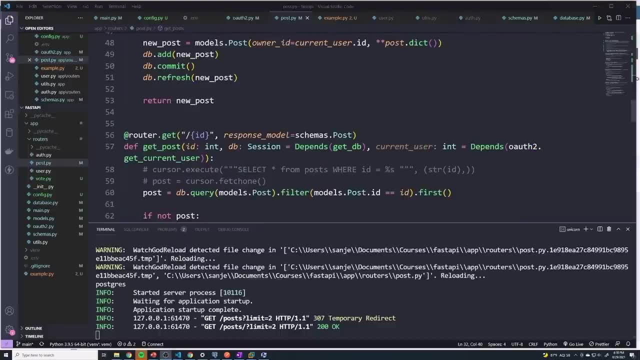 and then we're going to return post, like we normally do, send it one more time and it looks like everything is still working just fine, Perfect. So we finished the get multiple posts path operation or get all posts, And I noticed that we do have to go ahead and update the get. 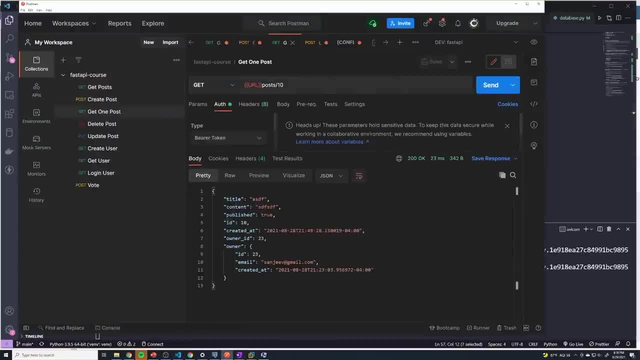 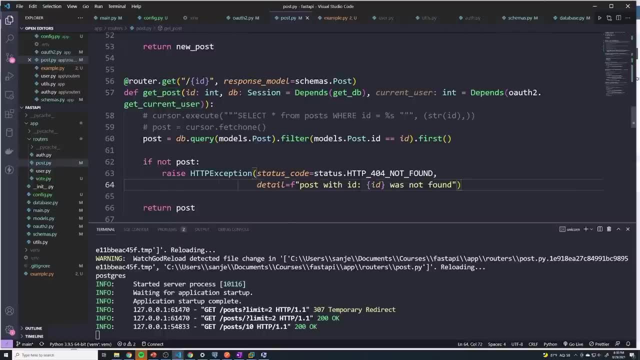 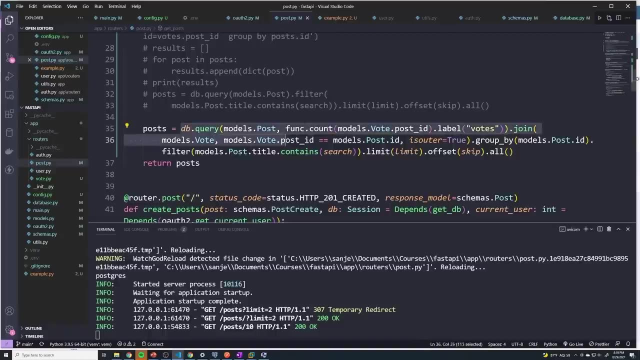 individual post, because right now if we go to get one post, you can see that we do not actually get the votes- vote count for that. So we definitely want to see that in here And we're going to have to perform the same exact join. So I'm just going to copy the previous query all the way up to: 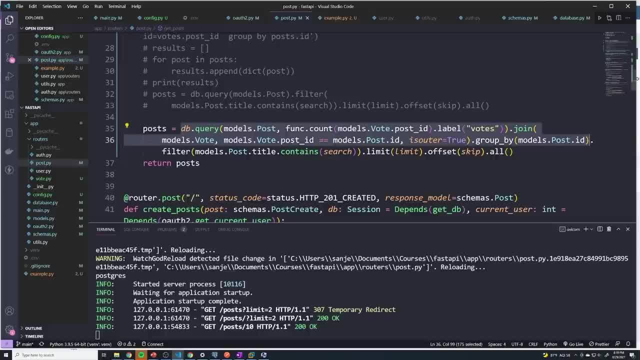 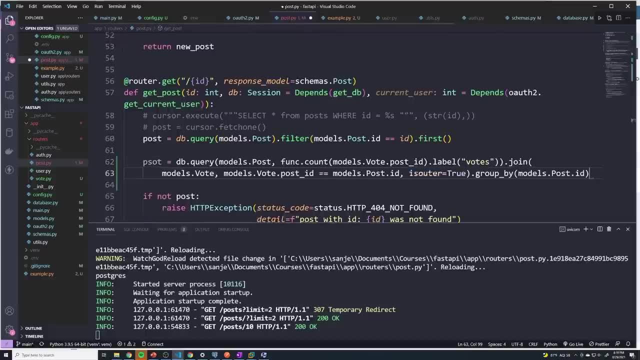 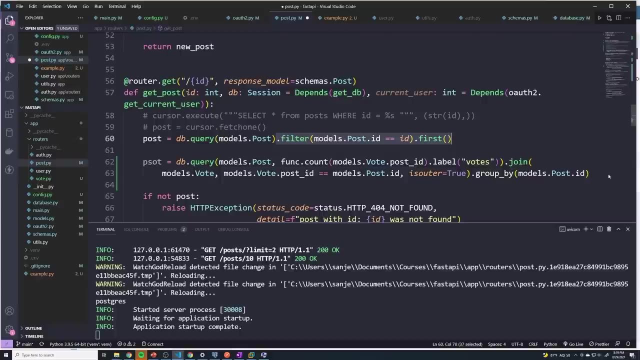 before the filter. So just copy that part, Say post equals, paste that in there And then we can filter. copy this filter at the end And that should ultimately get us what we want. I'm going to comment this one out. 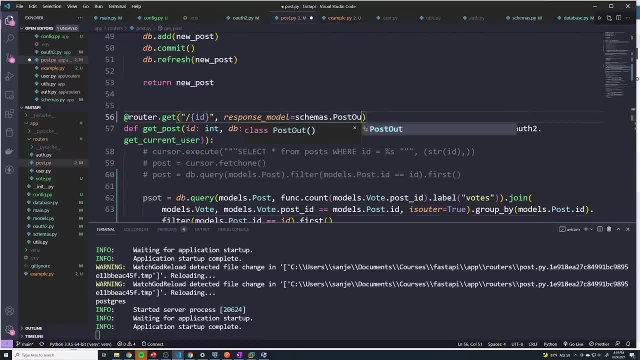 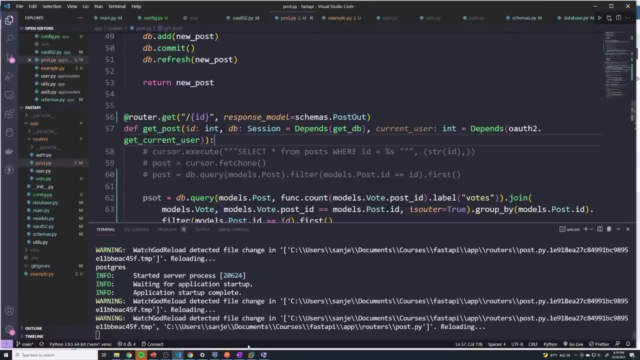 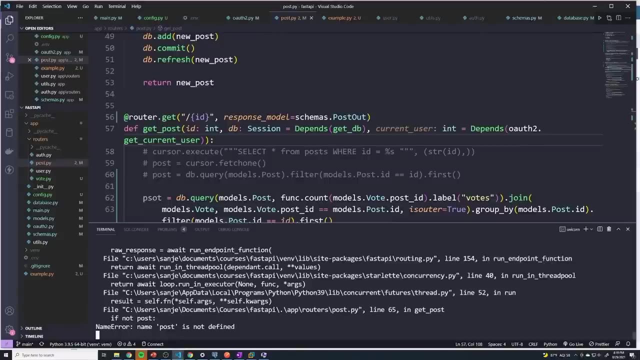 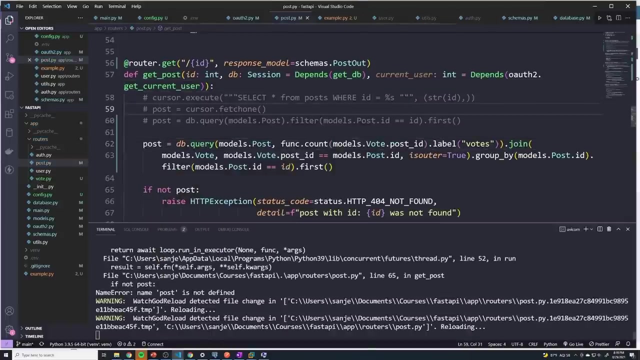 And keep in mind. we have to return post out instead of post now because we want the, the new format with the votes. But now if I hit send name, post is not defined. Oh, okay, misspelled that And looks like we fixed that. 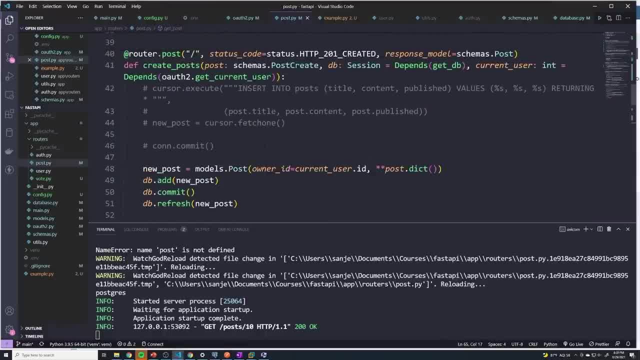 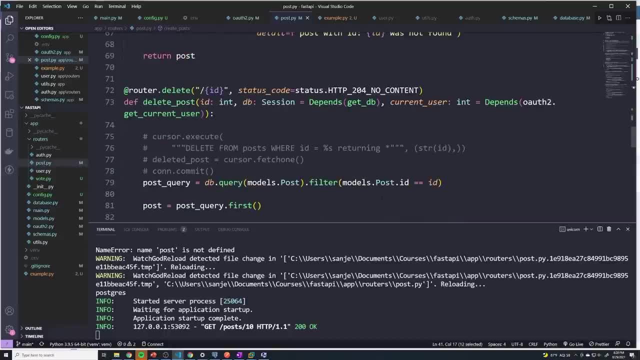 And then it's really up to you to see if you want to. you know kind of worry about creating posts and updating posts to make sure that you know when they create an update that they return the number of votes. but it's ultimately up to you. I think we don't need it in those. 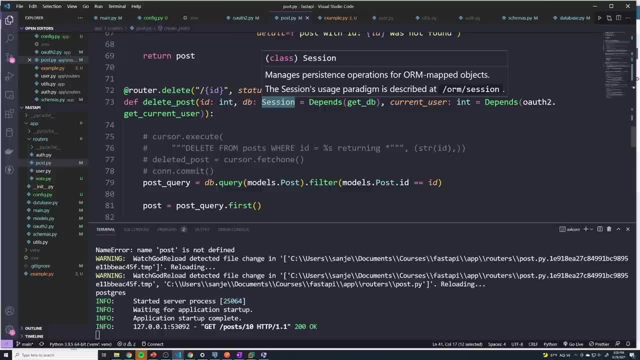 This more of just kind of returning back just the main information about the post, And then you know the queries for updating a specific post and then grabbing the votes gets a little complicated, So we're going to ignore that for the update And then we're going to go ahead and update that one. 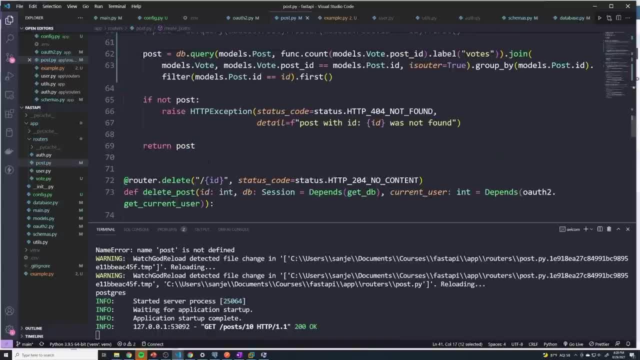 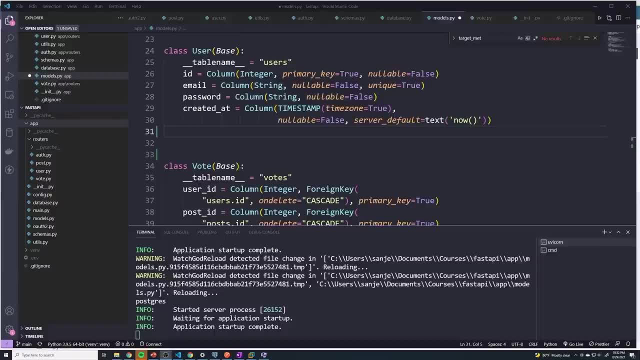 We're going to ignore that for the update and the and the create post functionality. Now, when it comes to building out the tables or the database schema, SQL Alchemy has a little bit of a limitation, And that is that SQL Alchemy doesn't allow us to modify tables. it doesn't. 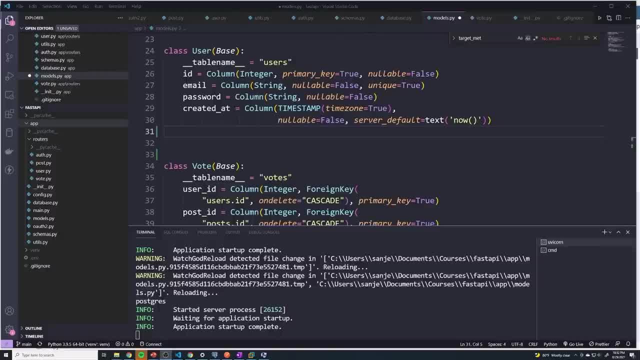 allow us to create extra columns, delete columns, add foreign key constraints. And that's because, when we define these models, what SQL Alchemy does is it checks to see if the specific table name are already exists in our Postgres database, And if it does, it's not going to touch it. So if we make 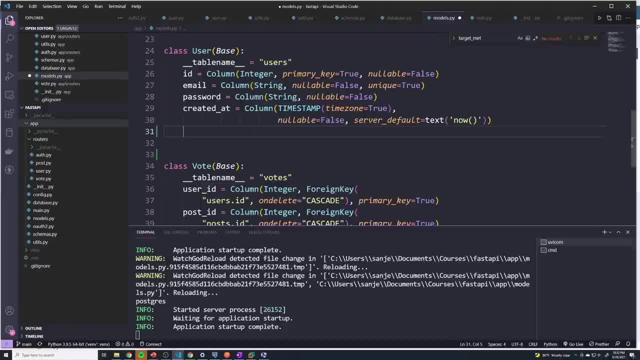 any changes, it will never push out those changes. It'll only create these tables if it doesn't already see a table with that specific name, And so we've had to resort to dropping all of our tables and then restarting our application. So that's SQL Alchemy builds it from scratch. 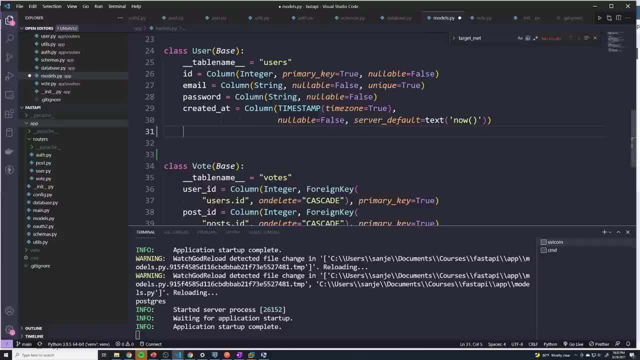 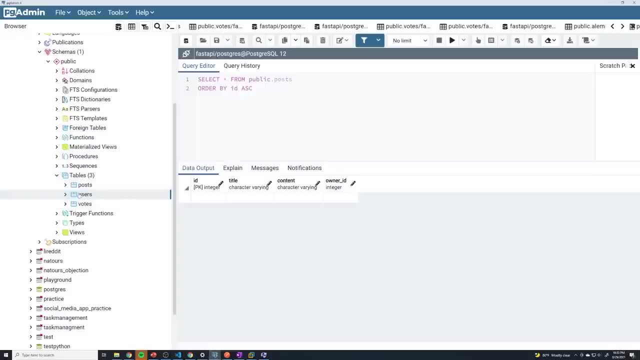 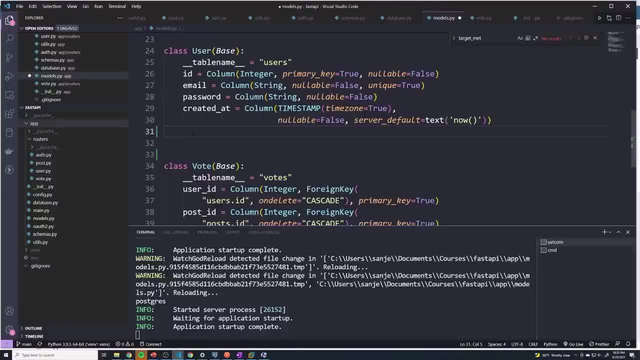 that we've got our three tables. Now, if I add a phone number class- sorry, a phone number column- to our user class, and I'll set this column to be just a string, And this is really just for demonstration purposes- you guys don't have to do this If I save this and reload this. 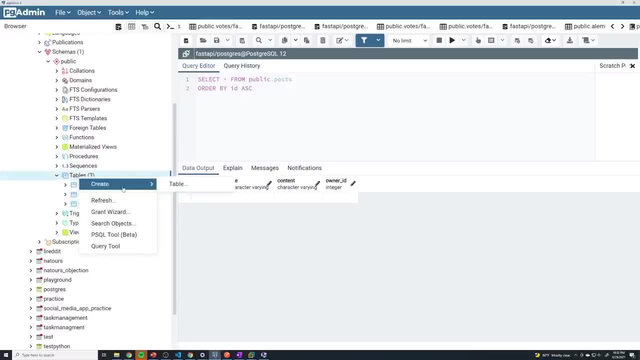 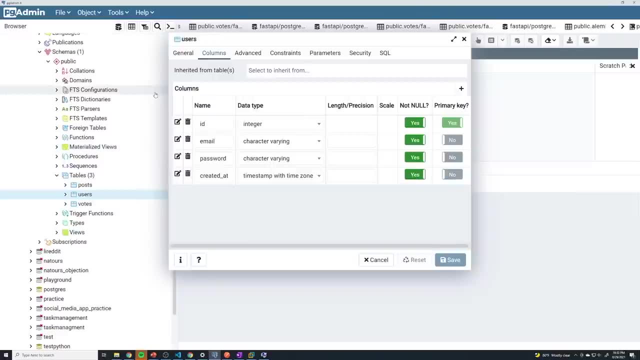 SQL Alchemy will not go into Postgres and actually create that column. If I refresh this and then go into users properties, you can see that it is not here, And so that's the limitation of SQL Alchemy. And so in this section, what we're going to do is we're going to take a look. 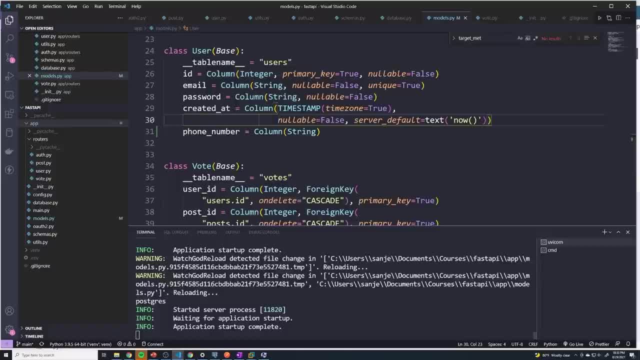 at another tool that will allow us to do a couple things. First of all, it's going to allow us to automatically update the columns based off of the models that we define here. So, moving forward, when we add this phone number column, it's going to automatically update our Postgres database. 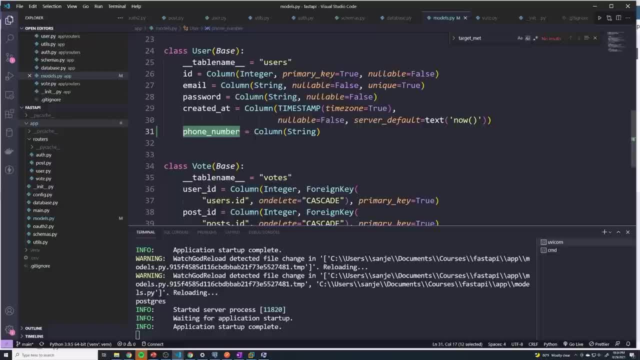 And this tool is called Alembic. It is what we refer to as a data database migration tool. However, it's much more powerful than that. It's able to allow us to, you know, create incremental changes to our database and actually track it, kind of like. 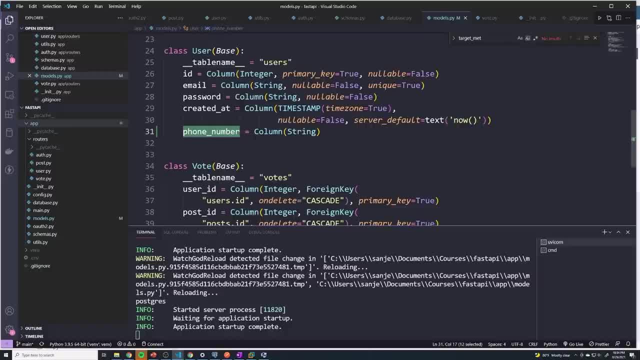 we do with code. So in the, in this lesson and in the next coming lessons, we're going to take a look at Alembic. we're going to see everything it has to offer And I'm going to hopefully get you guys at least a solid understanding of how to work with Alembic so that when you guys work on your 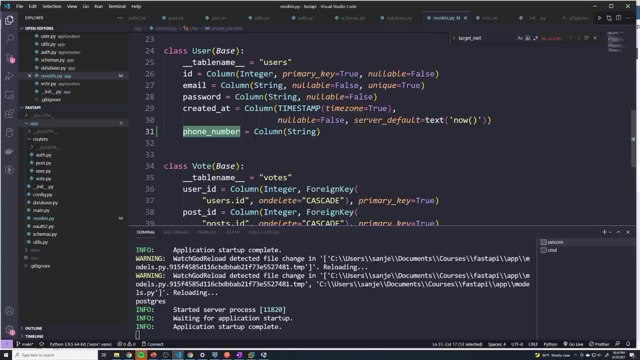 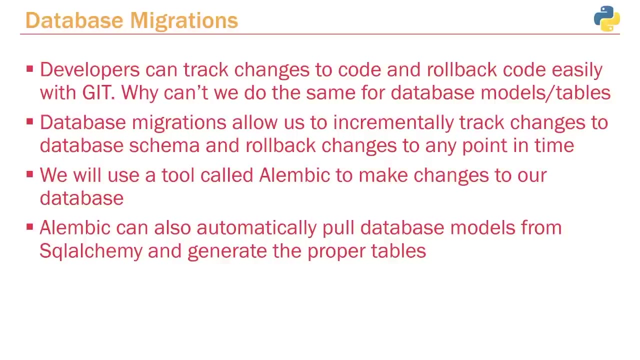 projects. you can immediately get Alembic installed, running and then manage your databases using Alembic, instead of having to either do it manually or use any other kind of unusual work around Now. one of the motivations for a database migration tool is came from the fact that 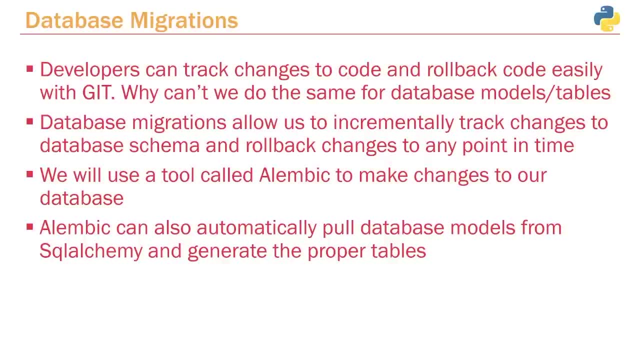 developers can track changes to their code and roll back their code easily with Git, And they wanted to be able to do the same thing for our database models and our database schema, And so they went about implementing what is referred to as database migration tools. 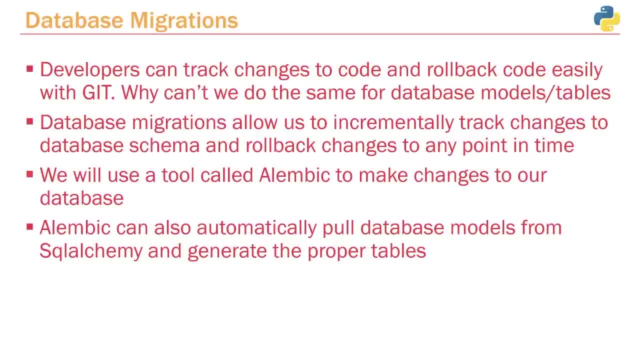 And so a database migration tool just allows us to incrementally track changes to our schema and roll back those changes to any point in time. And so as we go through our project, you know we kept adding new changes to our schema. And so as we go through our project, you know we kept adding. 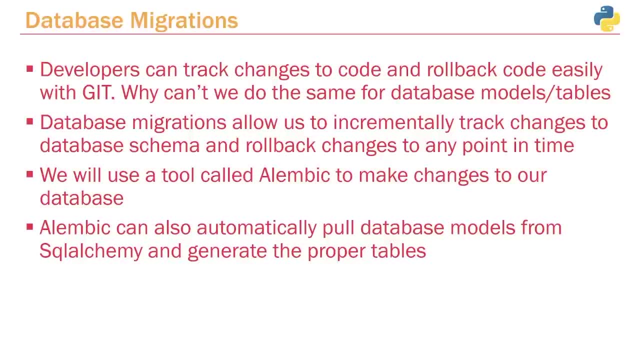 new tables and new features. what a database migration tool is? it's going to allow us to track those changes And so if we ever want to go back to a specific point in time so that we can kind of troubleshoot code at that point in time, it's so easy, it's just one simple command and 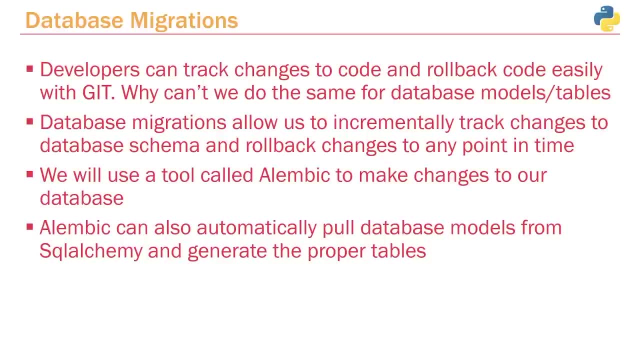 it's going to automatically update our database so that the schema matches what it was at that specific point in time, And so that tool that we're going to use, like I mentioned, is going to be Alembic, And what's great about Alembic is that it can also automatically pull all of the 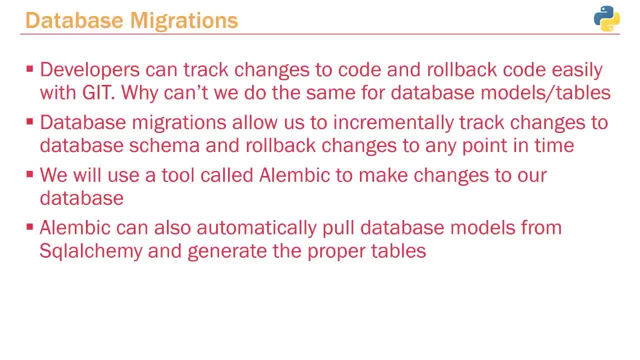 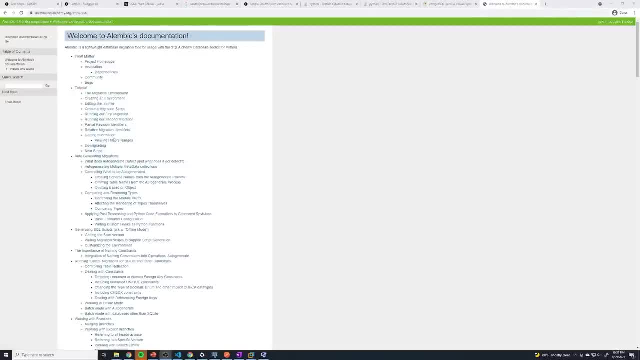 our SQL alchemy models and generate the proper tables based off of them. Alright, so this is the documentation for Alembic. So it's just alembicsqlcomorg, And if you want to kind of follow along, just select the tutorial right here, And this is just going to give you kind of a quick. 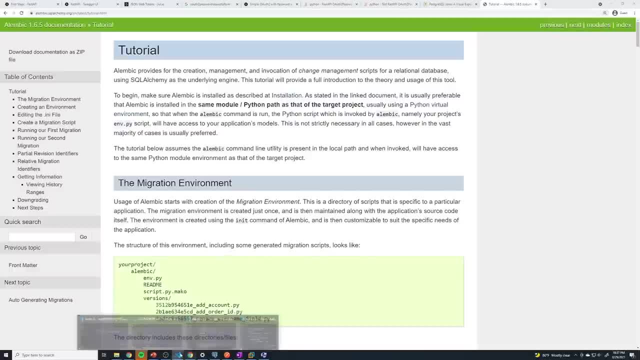 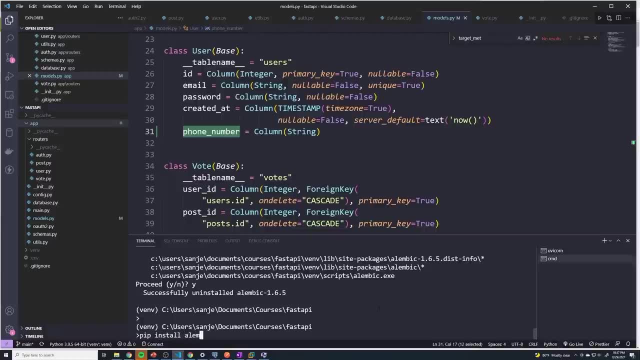 walkthrough of how to get Alembic set up. But I'm going to show you guys this so you don't actually have to follow the tutorial. So we're going to do a first of all we have to install the library. So we'll do pip: install Alembic. 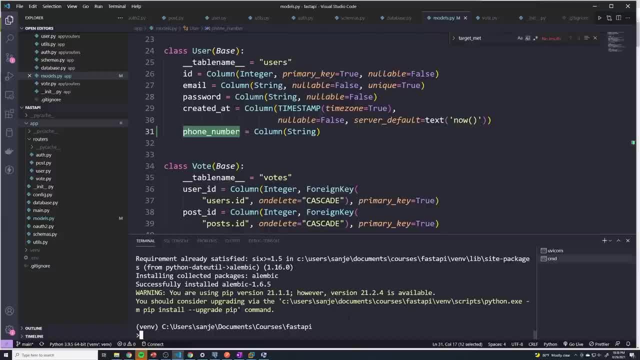 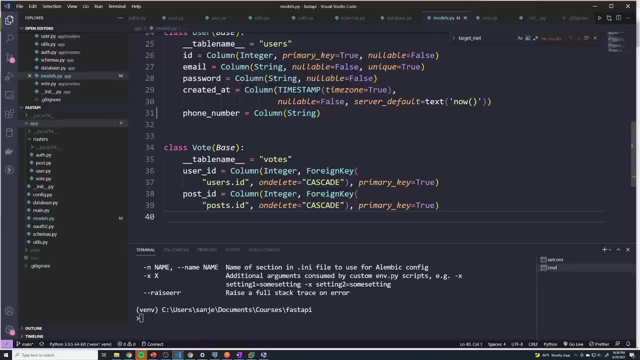 And so that will get Alembic installed And what it does is it actually gives us access to the Alembic command. So if I do Alembic dash, dash help, And actually, before we proceed any further, I want you to go ahead and delete phone number. we don't actually need that anymore. 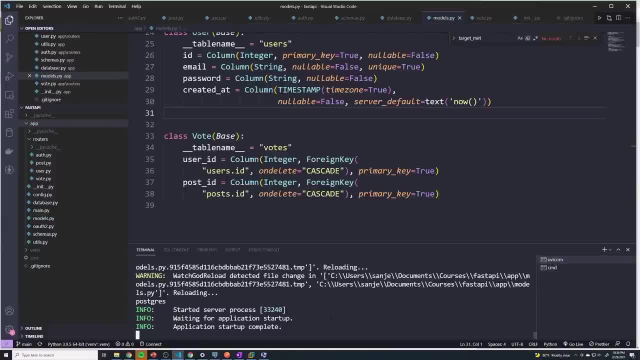 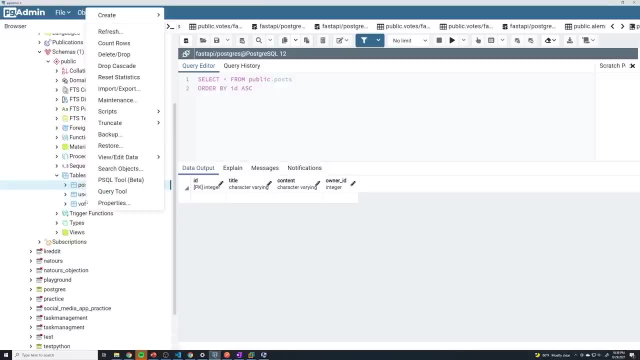 And then go to your app application and actually close that out, stop it so that it doesn't automatically restart for any other reason. And then also, what we're going to do is I'm actually going to delete all of our tables so that we can actually take a look at. 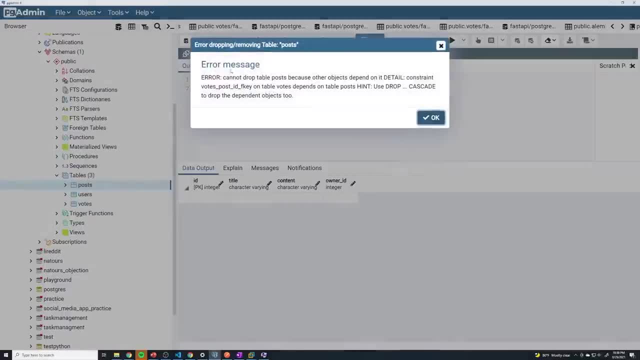 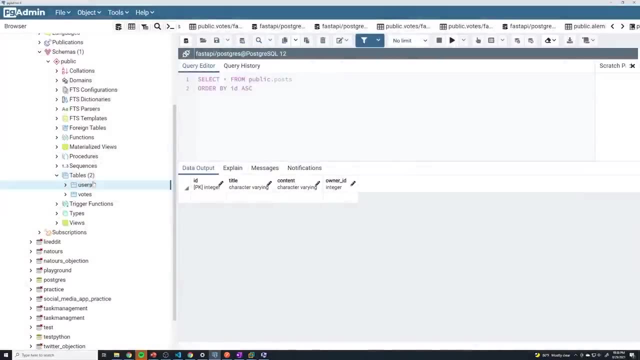 how this works. So do, delete, drop. And if you try to drop this table, it's going to say we can't drop it due to the foreign key constraint. that's okay, we can just do, drop, cascade, and that's going to delete it And we're just going to do that for all of them. 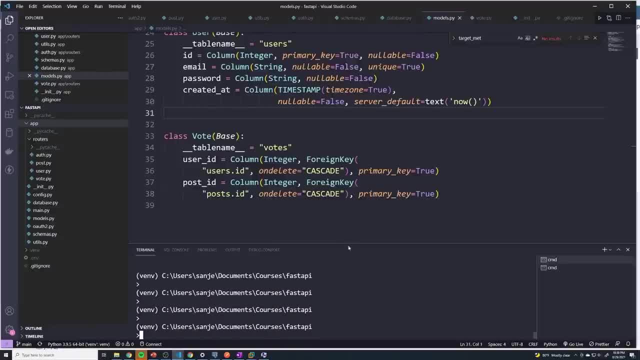 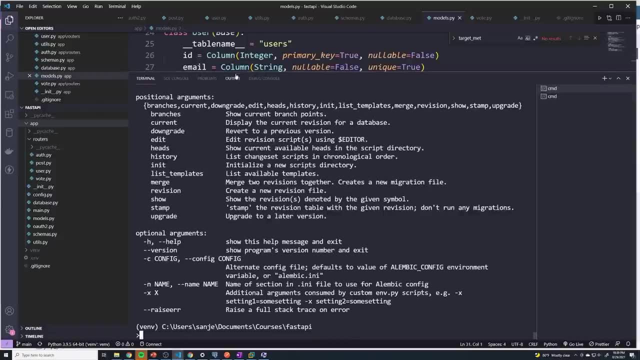 Alright. so now let's get back to Alembic. I'm gonna make this bigger for you guys, All right? And so we'll do Alembic dash, dash, help to see what commands we have. And the first thing that we have to do is we have to initialize Alembic, And what that's going to do is it's going to 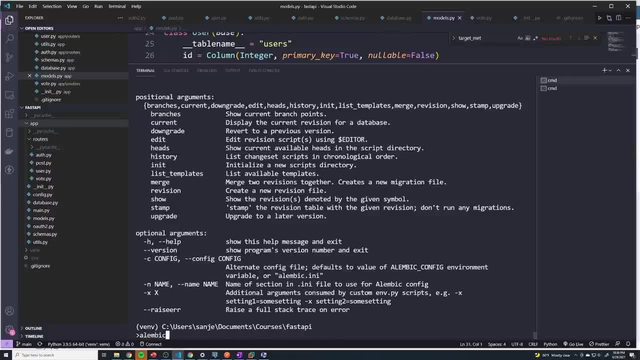 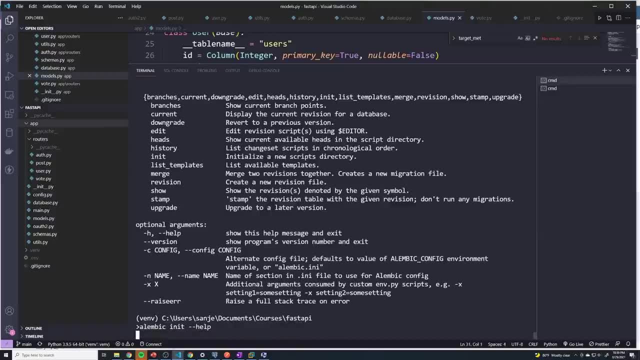 create an Alembic directory for us. So we'll do Alembic in it And then I'm just gonna do dash, dash, help to see if we need to pass in any extra flags, And then we have to give it a directory name. So when we run this command it's going to create a directory. I'm going to name the. 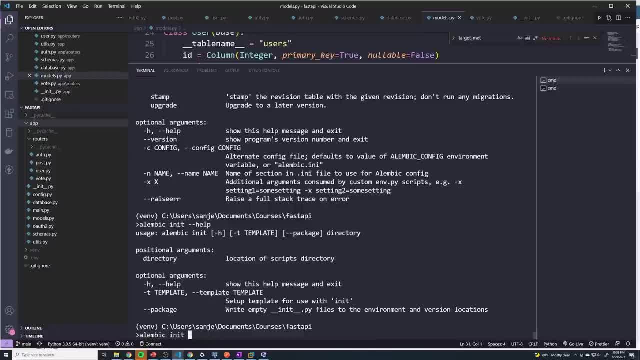 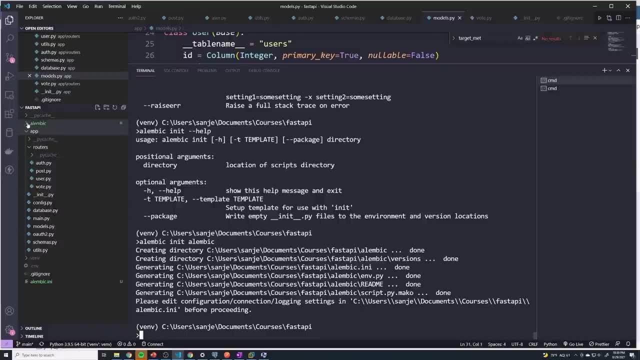 directory Alembic. You could call it DB database, whatever you want to call it, but I'm just going to call it Alembic. So it's going to create a folder called Alembic, And so you can see that we've got this folder called Alembic And notice how it gets installed outside of the directory. 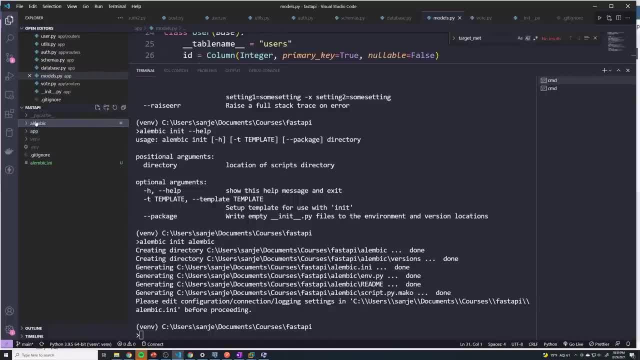 Of the app folder, which is what we want, And it also created this Alembic dot i and i file. So we'll take a look at both of those And the first thing that we want to do is go up into Alembic And there's really made one main file. it's the env dot py, So this is kind of like the 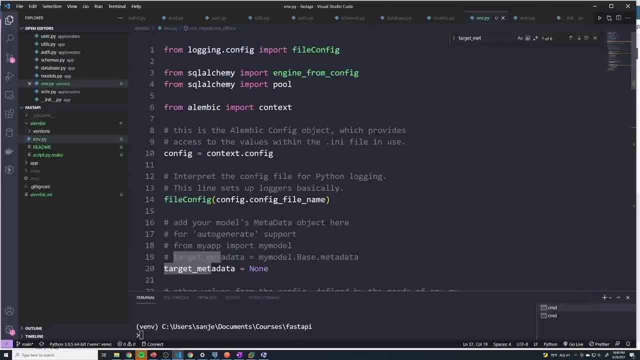 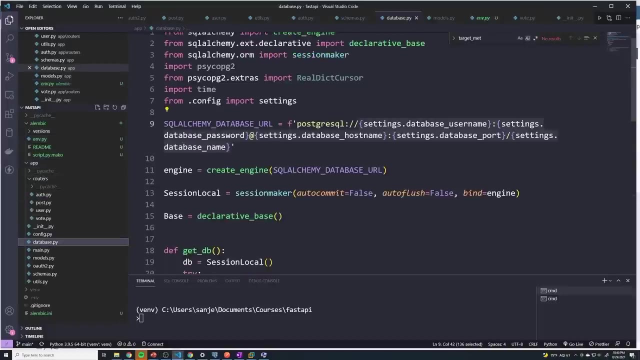 the King Kong configuration file And there's going to be a couple of things that we have to add to this file to make sure that things work. Because Alembic works with SQL alchemy and the models that you build with SQL alchemy, we need to make sure that it has access to our base, our base. 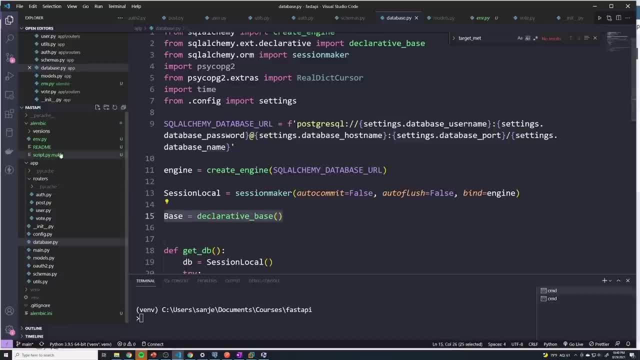 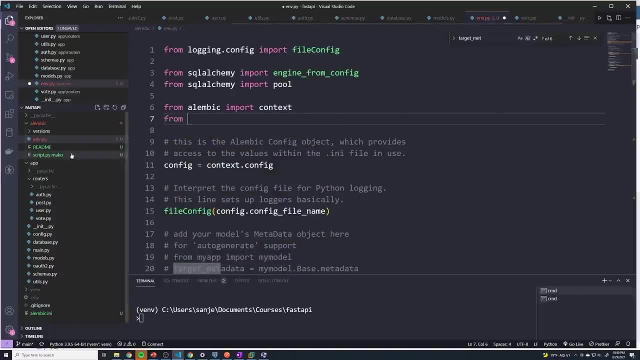 object right here. So we have to import this base object into the env dot py file. So I'm going to just go right here And we're going to say from: and what we're going to do is: how do we actually get to that database file, that that base object? we have to go into app And then we go into 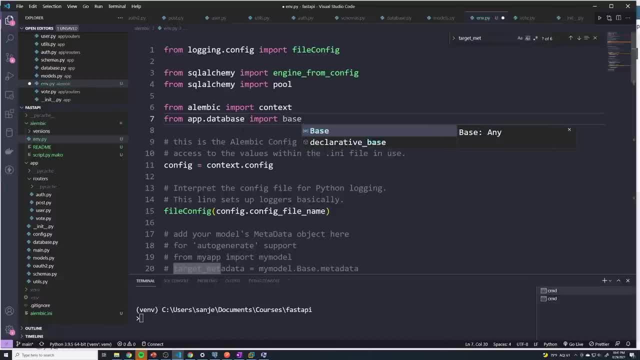 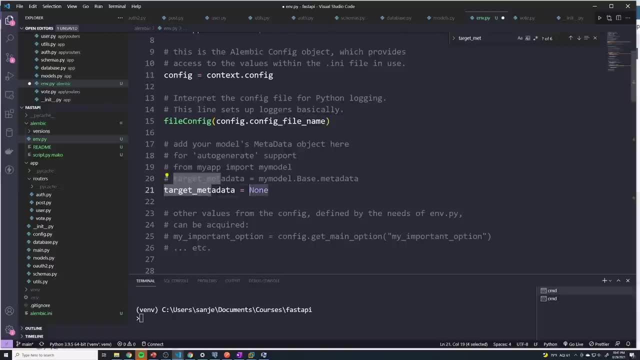 go into database and then we'll import base, All right. And so this is kind of give us access to all of those SQL alchemy models And then for target underscore metadata, instead of saying none, what we want to do is: we want to get base, So we're accessing. 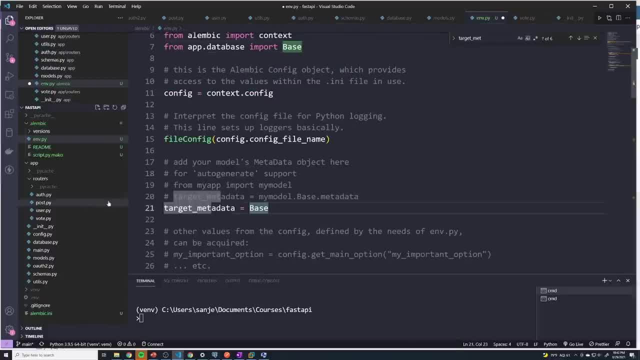 this should be a capital B. Actually, let's just double check that it's capitalized. Yep, it's capitalized here, So we'll go to base, and then we want to make sure we grab metadata. So that's all we have to do to rig this up to. 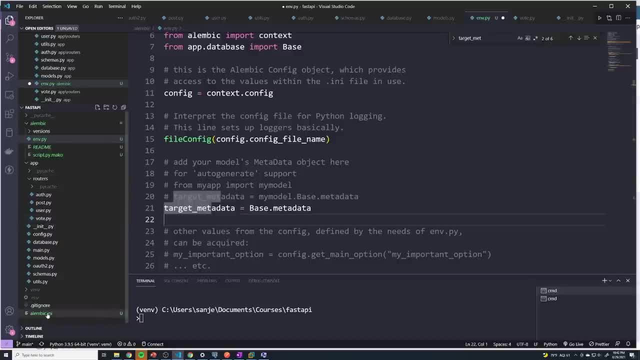 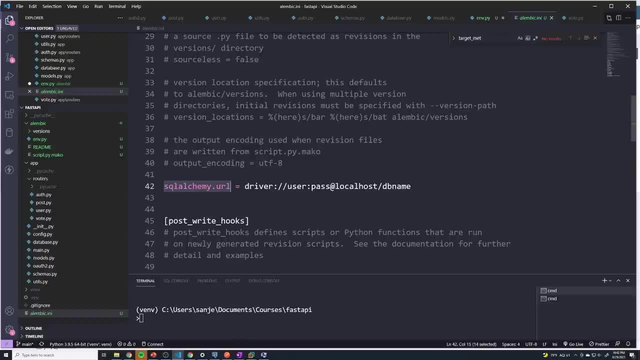 SQL alchemy. The next thing that we have to do is, if we go to alembic dot i and i, we have to pass in one value here, which is the SQL alchemy URL, which is basically what's the URL to access our Postgres database. And so just to show you what this is going to look like, 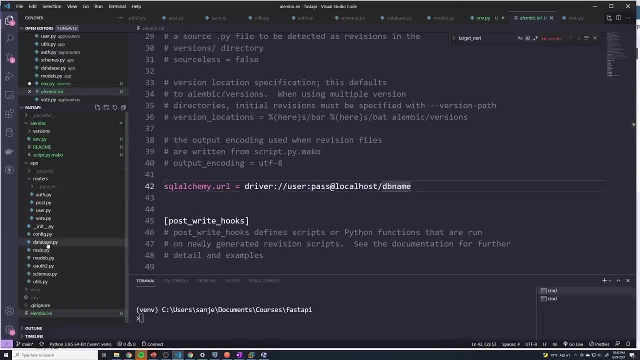 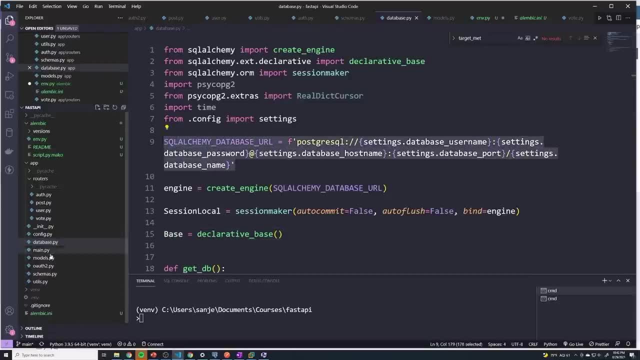 this is going to be fundamentally no different than the URL that we used within database dot py, which is this one right here, And so I'm just going to write this out. I'm just going to copy this first part right here, because I can never remember that. 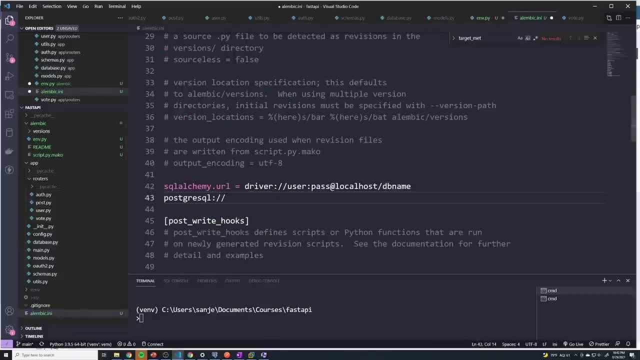 And so here I'm just going to copy that. So we say Postgres QL And optionally with the URL you can do a plus and then whatever driver you're using. So if you don't provide the driver, it's. 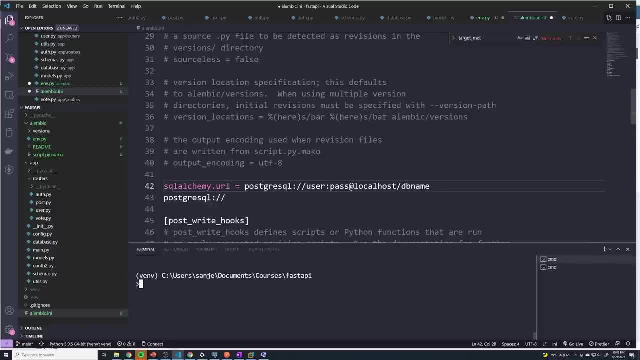 going to use whatever the default driver is, But we're using let's see which driver, what is our driver. So we're using let's see which driver, what is our driver. So we're using let's see which driver, what is our driver. 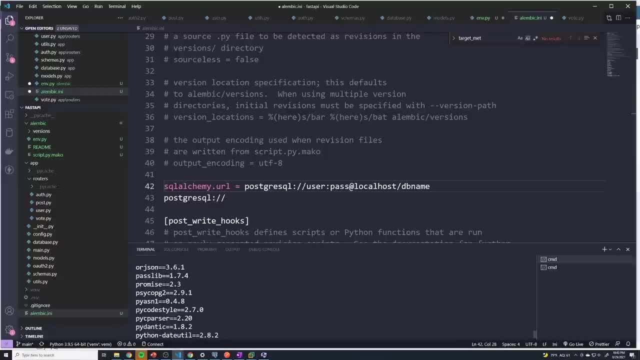 I do pip freeze, it's going to be this one right here. So this is the default driver for Postgres, So you don't actually need to provide it. But if you did, you could just say: plus PSY, co, PG, two. But like I said, it's the default one, So it's optional right. 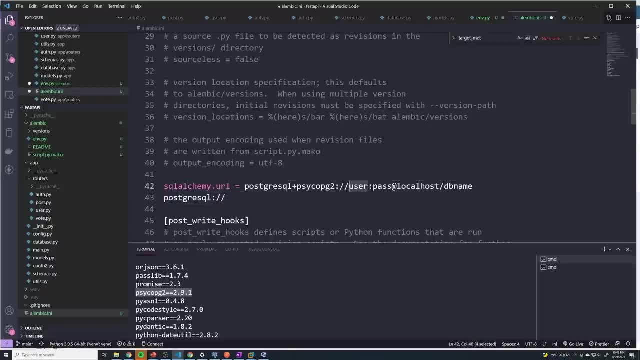 then we have to give it the username. So what's the username that's going to be using to log into your Postgres database? For me it's just Postgres. the password is going to be password 123.. It's going to be running on localhost And then, if you want to, you can provide the port. 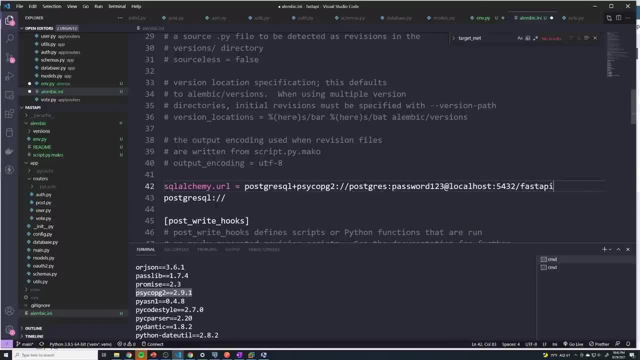 which is 5432.. And then your database name, which is fast API for me. So this is ultimately what the URL is going to look like And at this point, Alembic is set up and ready to run. However, you know, just like, just like we did before, I don't like the fact that we're hard. 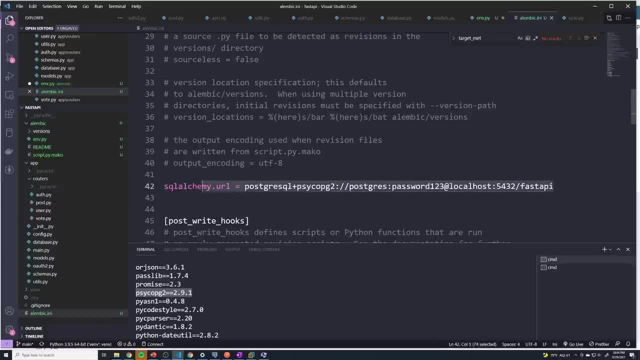 coding this data in here. It's gross. we're saving our password And if we move into our production server, it's not going to work properly because they're not going to use these credentials or this IP. So instead of doing this, 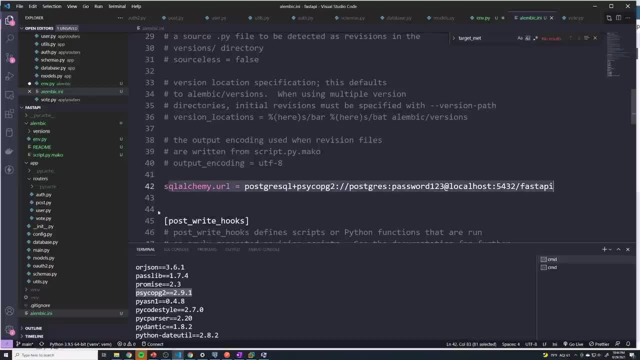 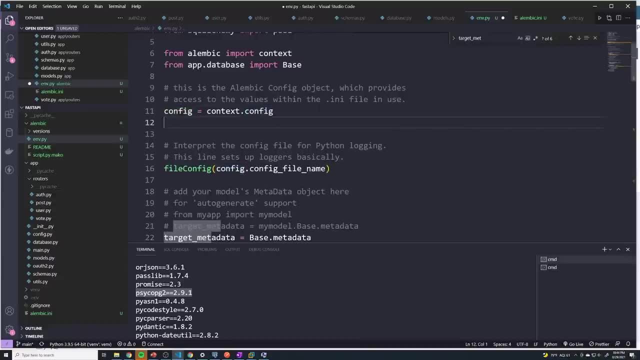 what we're actually going to do is we're going to override this value that's stored in this file, within the EMV dot p y file. And so under this config, right here, I'm going to set a new option. under the config object, I'm gonna say: config dot- set underscore- main underscore option. 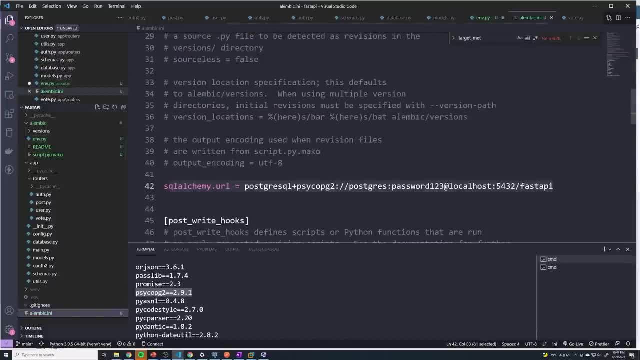 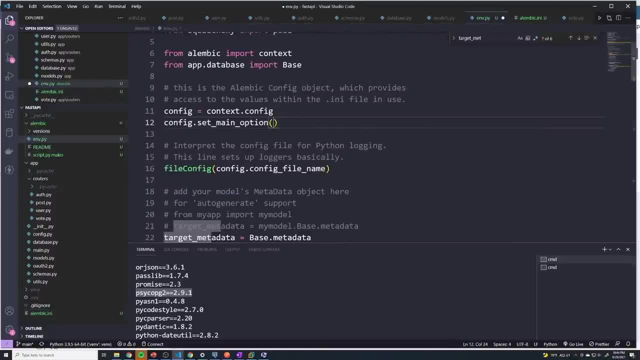 And here we can override any options that we have in here. So I'm going to override this SQL alchemy URL. So no matter what I put in here, we're actually going to override it. And here you just pass in a string, So SQL alchemy dot URL, So that's the value we're going to override, And then we're. 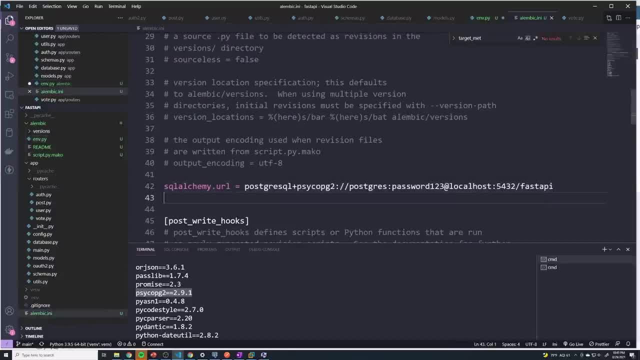 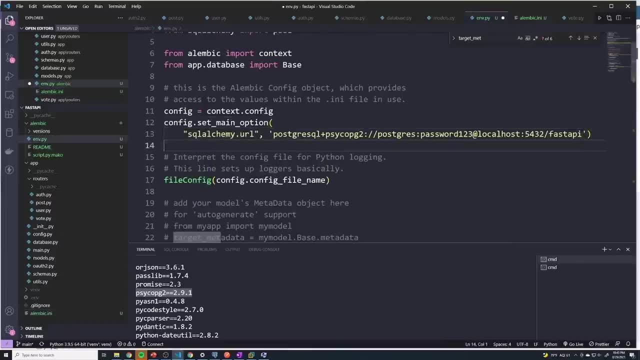 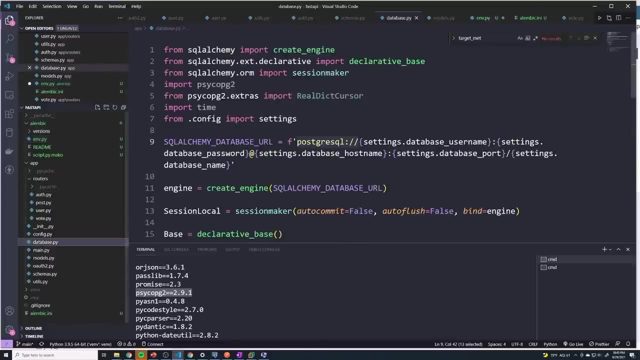 going to pass in our string, So I can just cut this out, And it's okay to just leave this blank here, All right, And so we've hard coded the string here. So we haven't technically fixed anything. But what we're going to do is just like we have in our database, dot p y file. you can see. 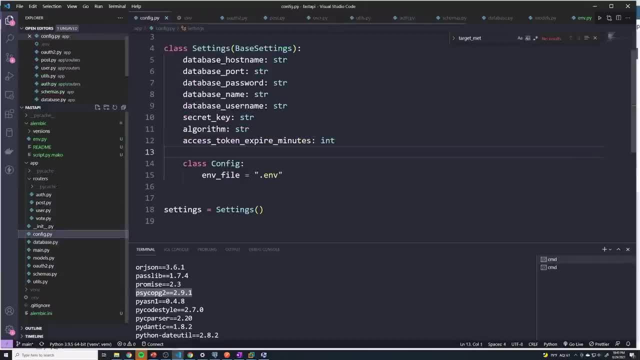 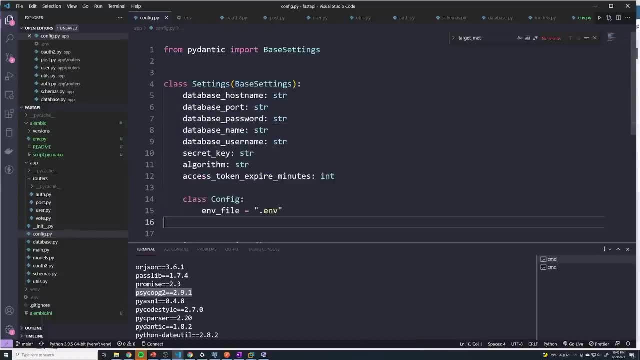 that we have the environment variable, And that's going to be the same thing we did with the main object. Right, that comes from our config file, which is making use of this pydantic class where we can grab it from our environment variable, And so what we're gonna do is we're. 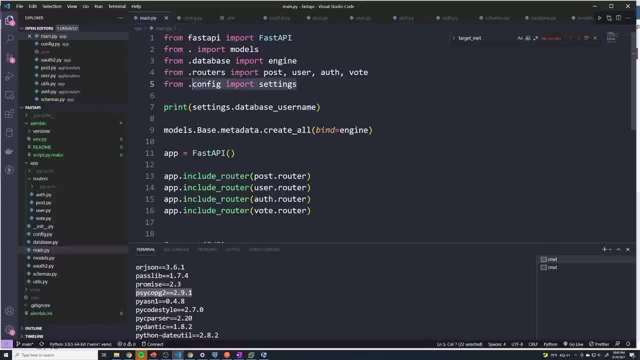 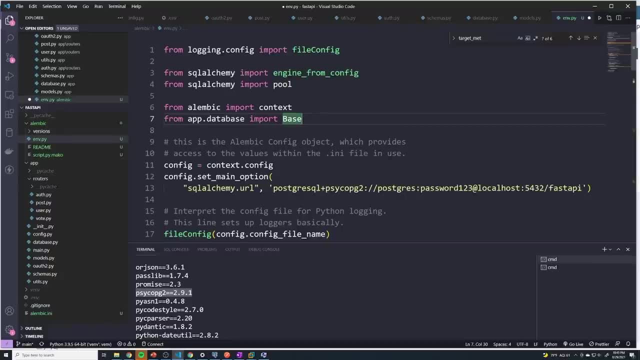 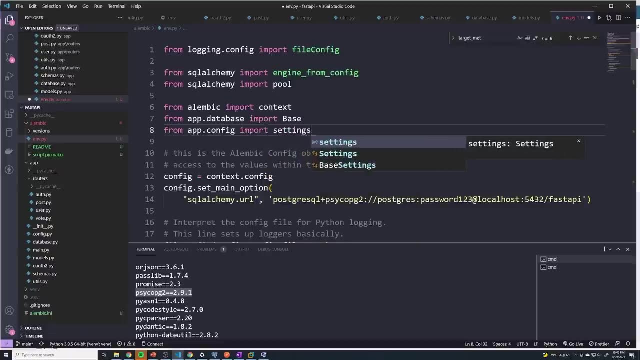 going to do the same exact thing we did with main right: we imported settings and we're just going to do that in our EMV dot py file so we can access all of our environment variables. So I'm gonna say, from app dot config import settings. And so now 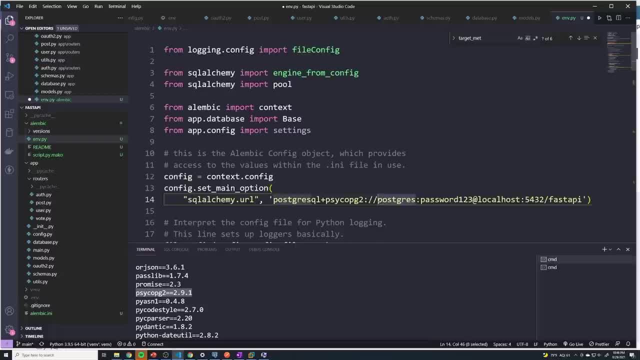 I have access to the settings object. I can override all of these. So this is going to be the username. So I can say settings dot username- And actually I don't think that's what it is, It's database underscore username, And then we'll override the password, which. 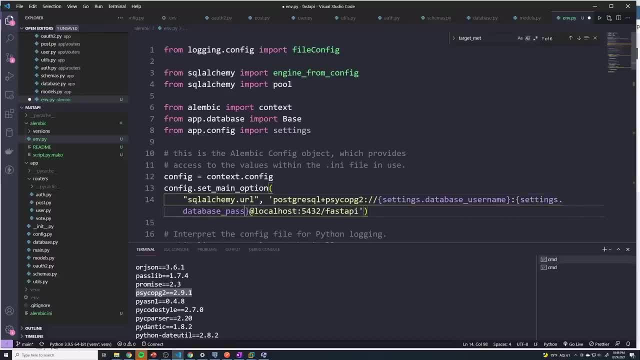 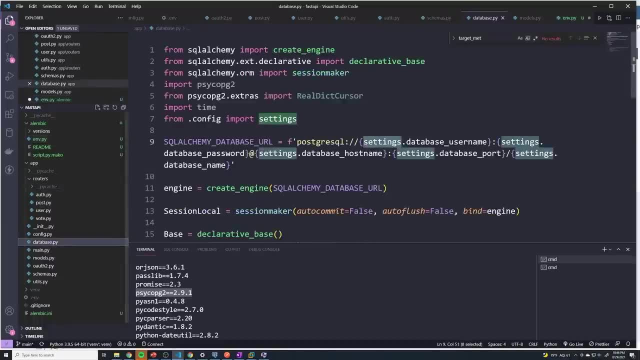 is settings- dot database, underscore password. And in reality, instead of just typing this all out myself, we actually have this written out in our database dot py file, So I can just copy this here, And that way we don't waste too much time. 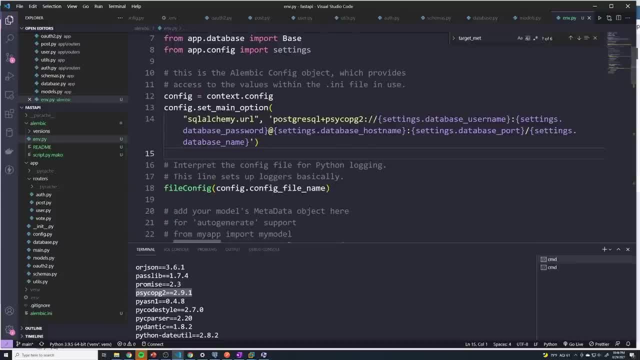 Okay, so we've got our URL set and we're not hard coding any values And at this point- this point- Alembic should be set to actually connect to our database and modify any of the tables, generate tables and be able to really perform any actions that we wanted to moving. 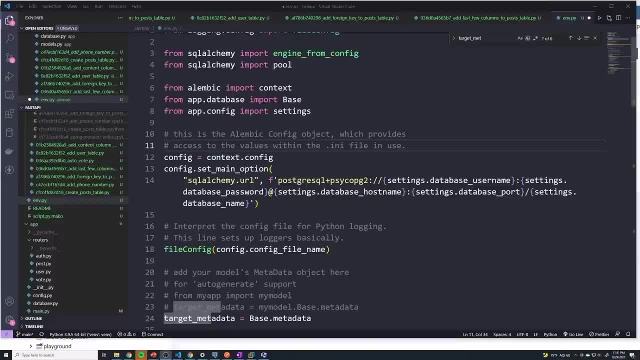 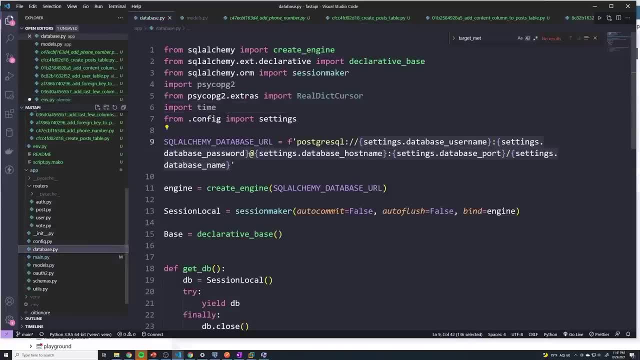 forward. Hey guys, I made one tiny little mistake. If you take a look at where we're importing base, I wrote app dot database And if we take a look at that, it looks like we are grabbing our base right here. But this is not the one we want. Instead, what we want to do is we. 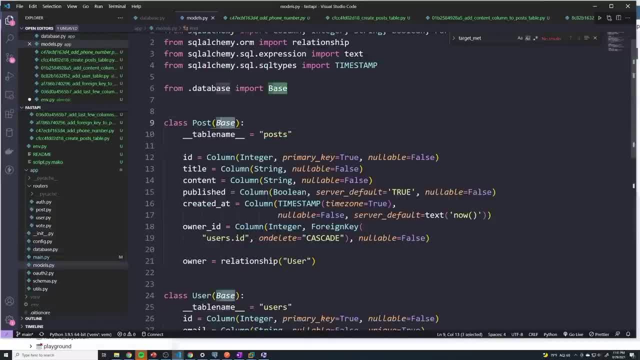 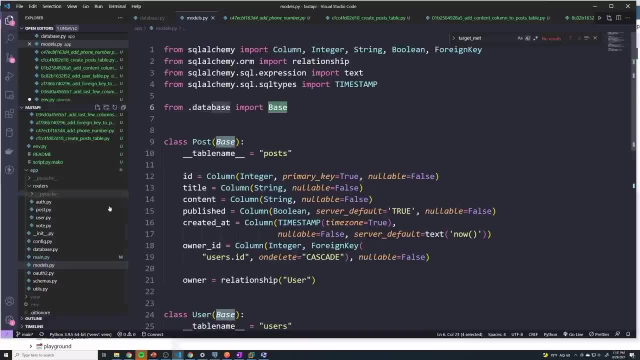 want to import it from models, So we want to import base, which is technically getting imported from that same file. But by doing it from here it'll allow Alembic to read all of these models, And if we do it directly from database it's not going to work. So what I want you guys to do is 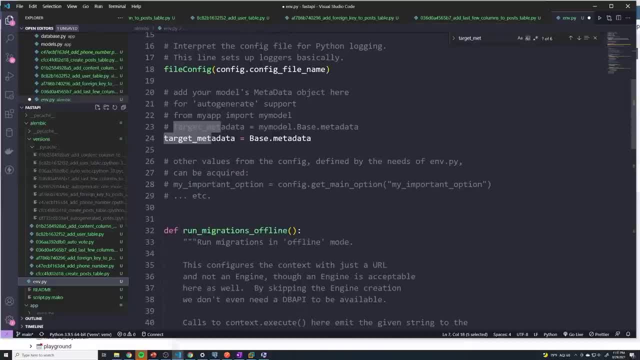 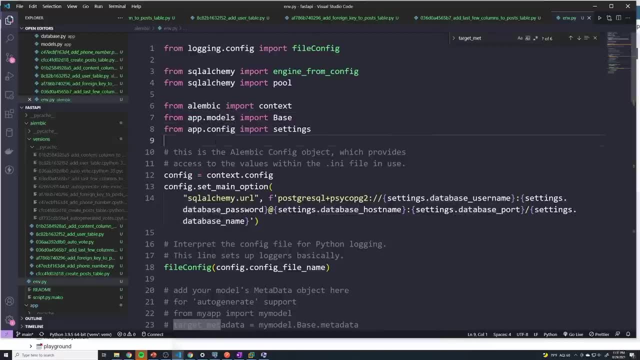 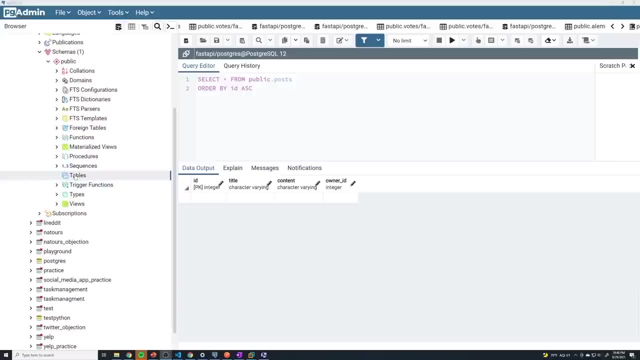 go to your env dot py file And just change this from app dot database to app dot models, And that should fix any potential issues that you could have. Okay, so you just to quickly recap. we have cleared out all of our tables, So there's nothing in our 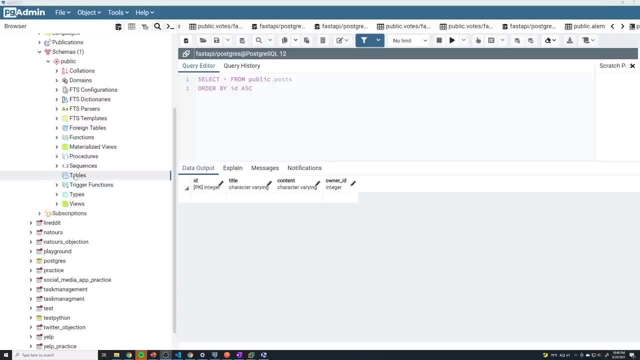 Postgres database. we don't have any tables defined And we're going to do this all through Alembic. But what I want to do is I want to kind of go through this like we would have if we had already known about Alembic from the start of our project, And so we're going to take this step by. 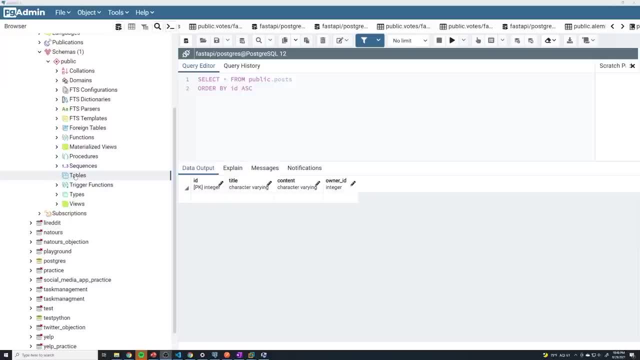 step right, Because when we first started creating tables in our Postgres database, we kind of went along with what we were working on in our app. So the first thing we did was we created a post table, And that's because we didn't learn about how to actually create users. we didn't learn about hashing. 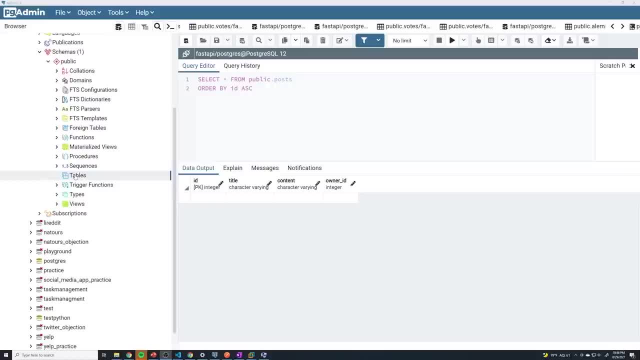 passwords. we haven't gotten to the user section, So we originally just had a post table with a couple of fields And then, after working through our code, once we've finished all the CRUD operations for posts, we then learn how to register users, And at that point we had to create a table. 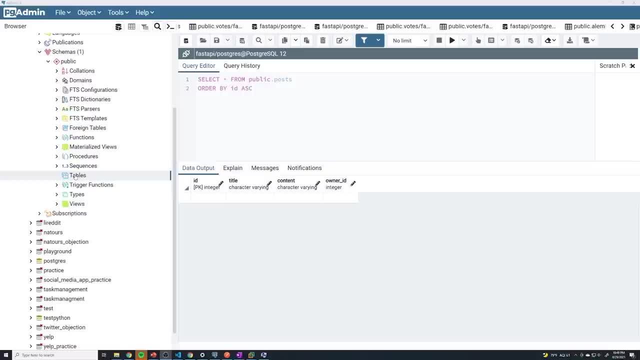 for users. And then after that, the next logical step was: Hey, how do we set up the relationship between posts and users? then we have to modify that and set up the relationships, But first we a foreign key And then finally, after that, the last thing that we had to do was we created 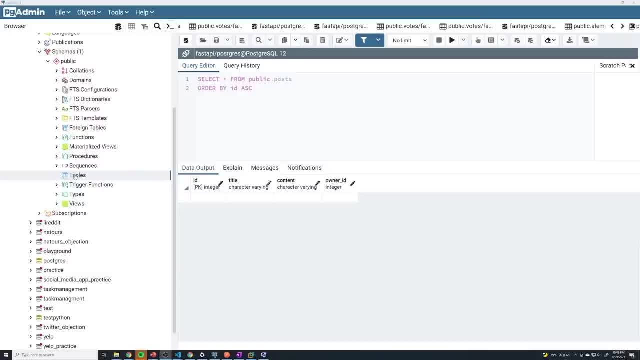 a voting table or a votes table, And then we set up all of the necessary foreign keys for that. So we're going to- so we're going to do this step by step, just kind of like how we did it with our our project. But we're going to do this with the database, so that 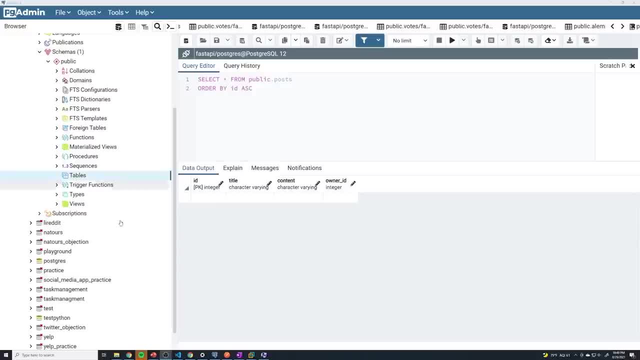 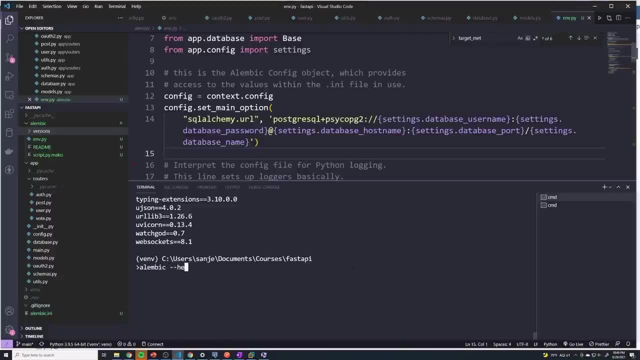 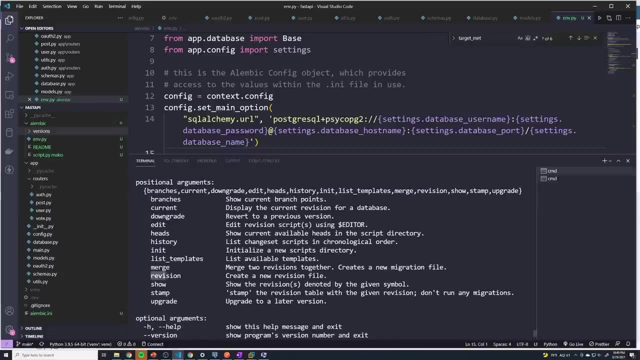 you can see how we would have done it if we had already known how to work with Alembic. Alright, so first things first, do Alembic, Alembic, dash dash help. just to see what commands we have, And so there's a few different commands, But the first one that I want to focus on 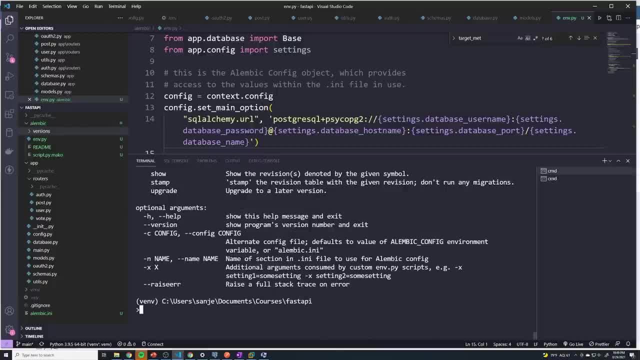 is revision. So when we want to make a change to our database, we create a revision. So the revision is what really tracks all of the changes that we make on a step by step basis. So we're going to do Alembic revision- dash, dash, help. And then we're going to do: 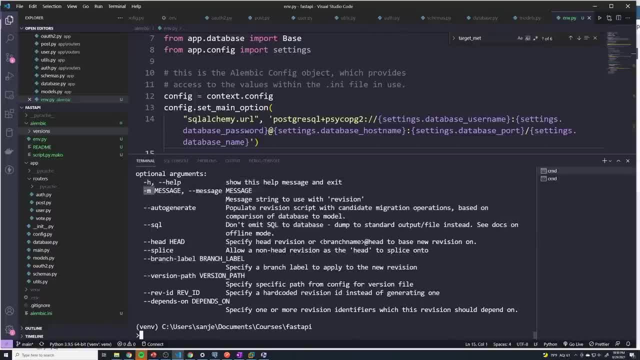 revision And we'll see the different options that we have in our disposal. The first one is that I- really the only one that I care about- is the dash M flag. So it's kind of like when you do a get commit, you can add a dash M a message, so that you can kind of 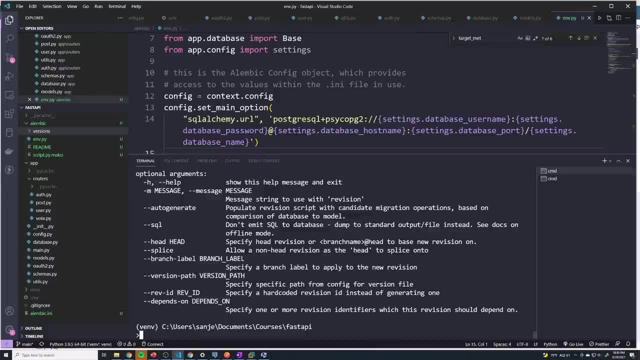 have a human readable name associated with each revision. So I'm going to say get sorry, not get Alembic revision dash M and I'm going to say this is going to be create post table. So this revision is going to be responsible for. 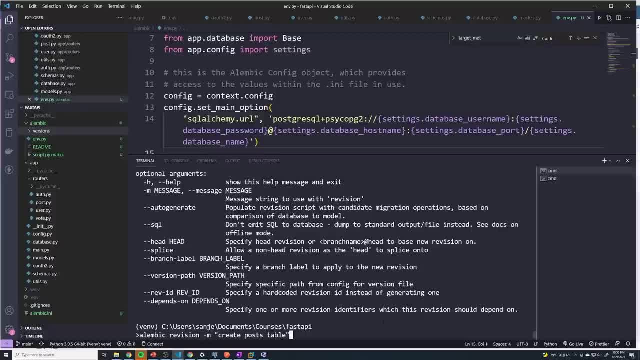 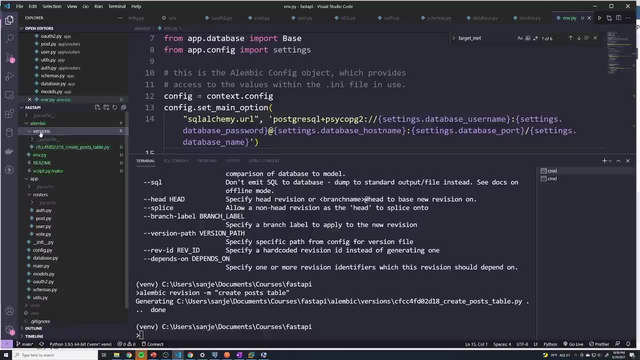 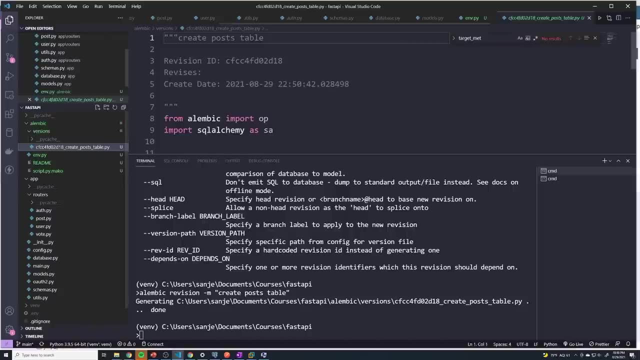 creating a post table. We'll run that And I want you to notice something right, you can see that it created this file under the version. So the versions folder under the Alembic folder is going to contain all of our changes And if we take a look at the 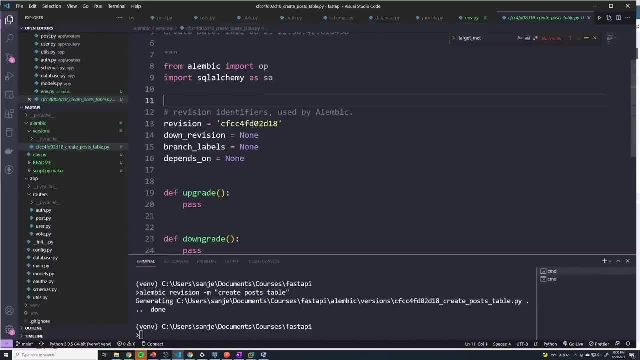 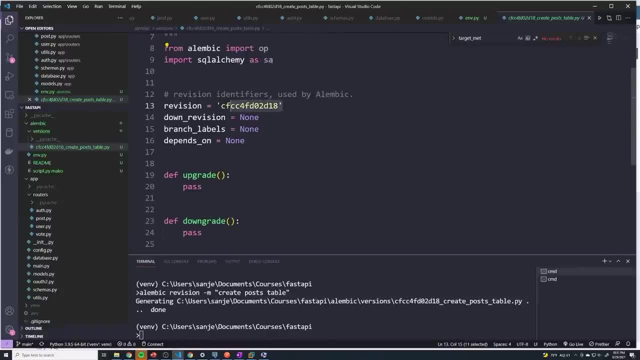 revision. there's a couple things to note. So you'll see that we import OP from the Alembic library and then we import SA from the SQL alchemy library And then you can see the revision ID that it gives it, And then there's going to be two different functions that are empty at the moment. So 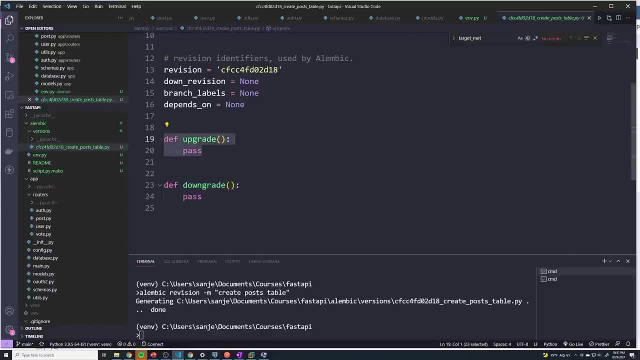 these functions are pretty important. What they are is the upgrade function. when we run the upgrade, what it does is it runs the commands for making the changes that you want to do. So in this case, we want to create a post table. So what we're gonna do is we're. 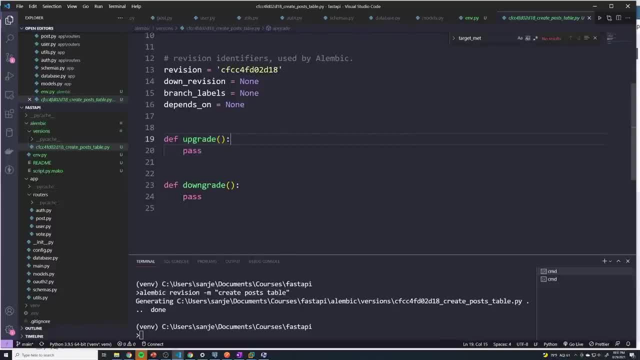 going to put all of the logic for creating a post table within this function And then if we ever want to roll back right- if maybe I create the table and I realized I've messed it up and I don't want it anymore, then we have to put it in all of the logic in the 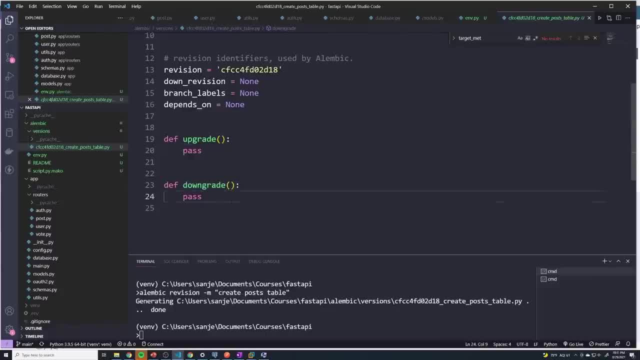 downgrade function to handle removing the table. So the upgrade just handles the changes And the downgrade handles rolling it back. but it's all manual. you have to define how to do all of that. So let's go ahead and set up the upgrade function And let's configure. 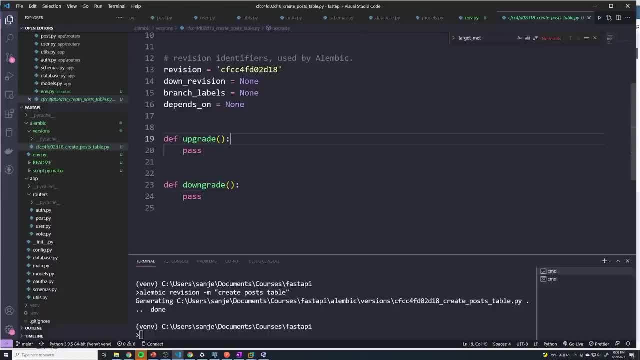 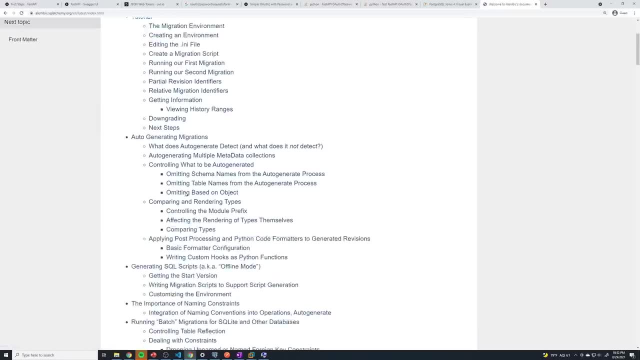 all of the necessary columns for our post table. All right, And if you ever want to take a look at the documentation for this, what you want to do is select documentation here And then you want to go down, down, down, all the way down to API details And 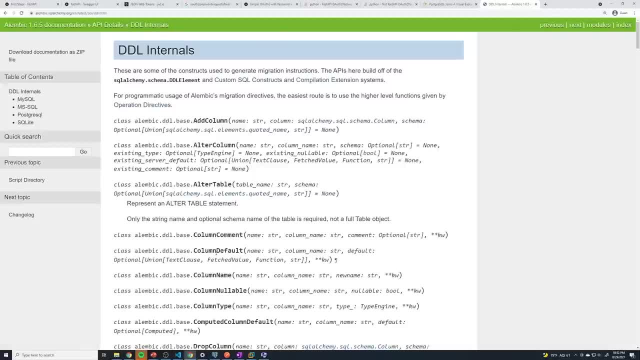 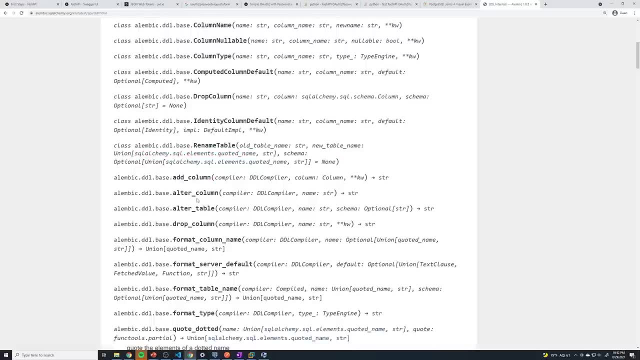 you want to go to cdl internals. So this is going to show you how to actually perform the various operations. So, if you want to create a column, if you want to add a column, this is the command that you're going to run. If you want to alter a column, if you want to modify a table, drop. 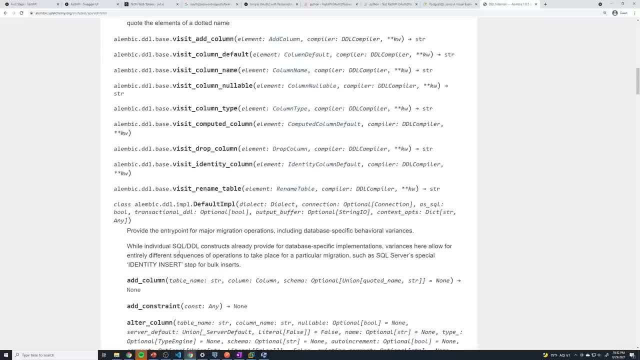 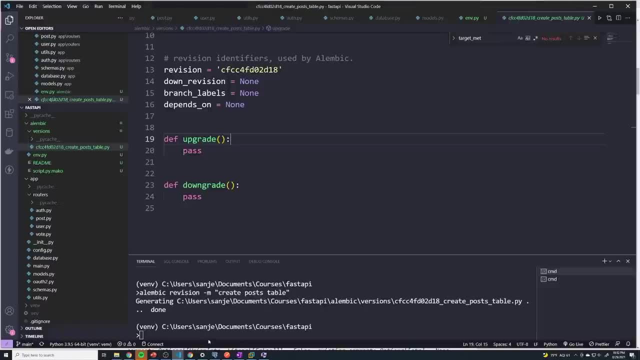 a column, create a table. all of these are all listed here, So this is the sheet that you're going to reference on a fairly frequent basis when you're working with Alembic, because I can never remember each of the things, But we're going to go ahead and create our post. 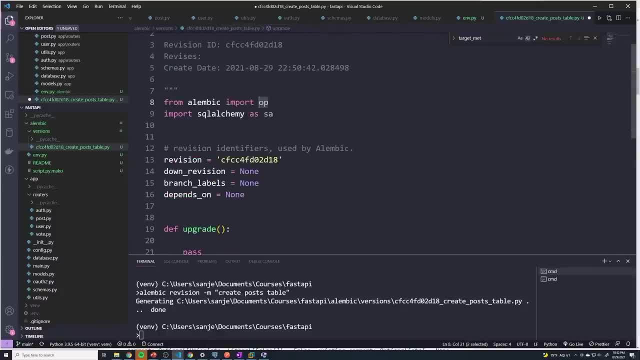 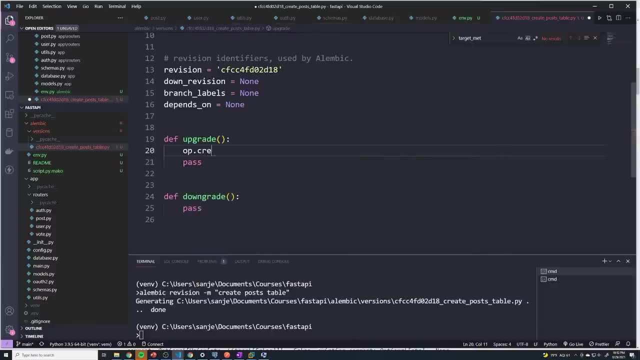 table And so we access the OP object from Alembic. I'm gonna say OP And then, if you look at the documentation, the way to create a table is you do create underscore table And there's going to be a couple of properties we have to pass in. So what's the name of the table? 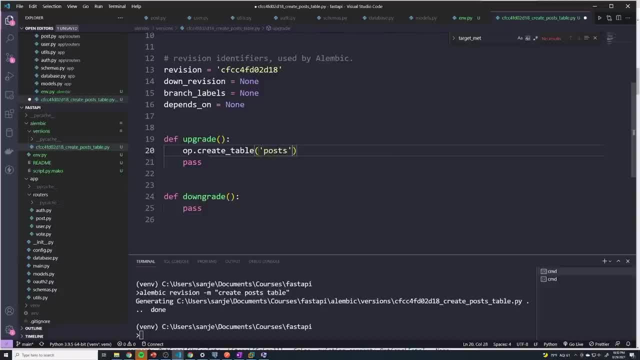 in Postgres. Well, we're going to call it posts, And then we have to define our columns. And I'm not going to do all of our post column because it's going to take a little bit of a while And we might do it later on, But we're just going to define two columns. So 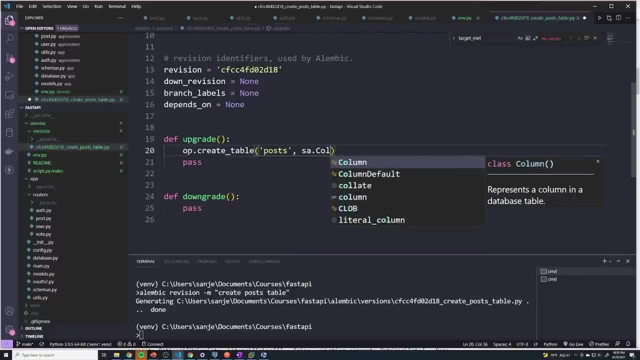 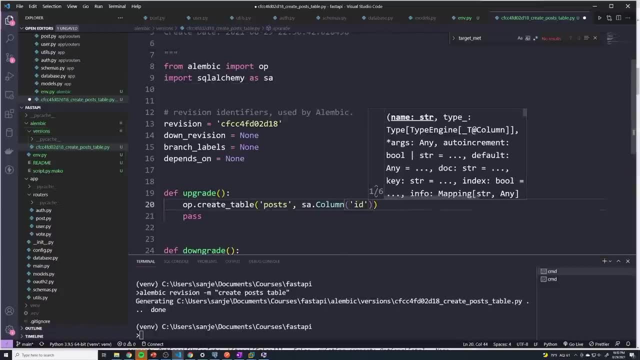 the first one is going to be. Well, first of all, we do essay column, So we're grabbing the SQL alchemy object, And so this column is going to represent the ID. the name of it's going to be ID, it's going. 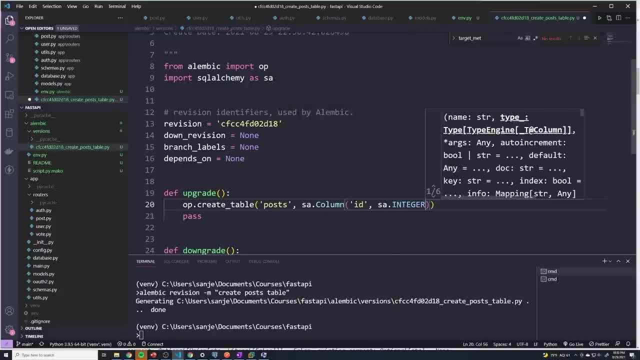 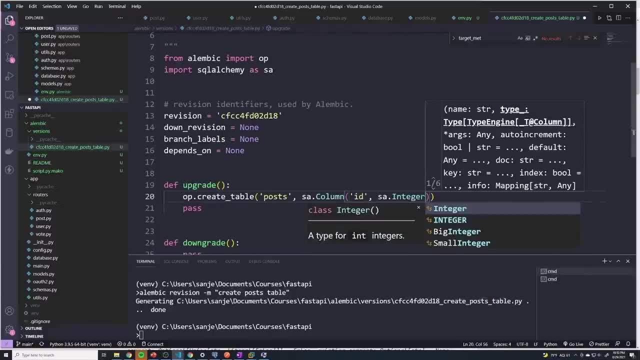 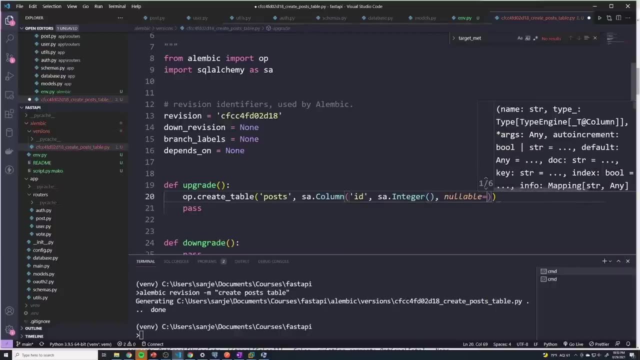 to be a type of integer. I may have accidentally imported Nope, that were good integer And then we can set nullable equals false, Which means it's required. So I'm going to put in my type of items. These are the elements. 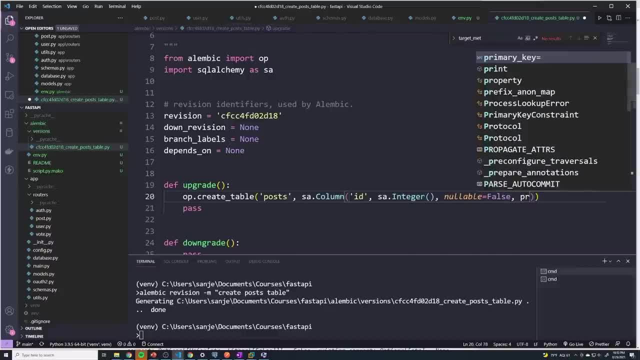 I'm going to set nullables equals false, which means it's required, And then I'm going to do this item as well, And then we also want this to be the primary key. So you just do: primary key equals true. All right, fairly straightforward, right, guys? so we can then go in and create a second column. 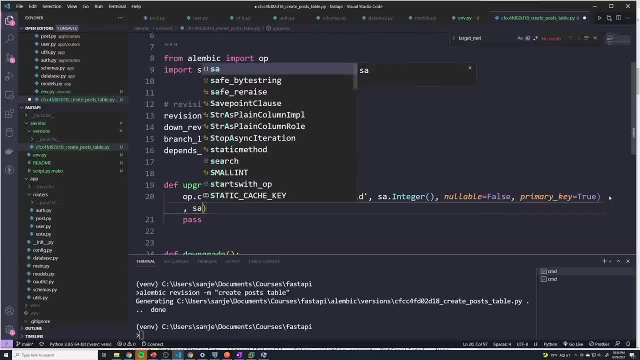 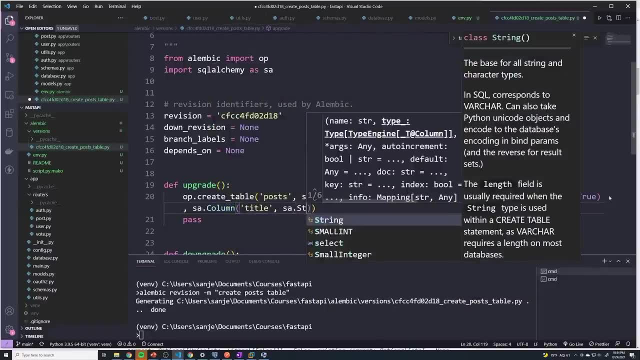 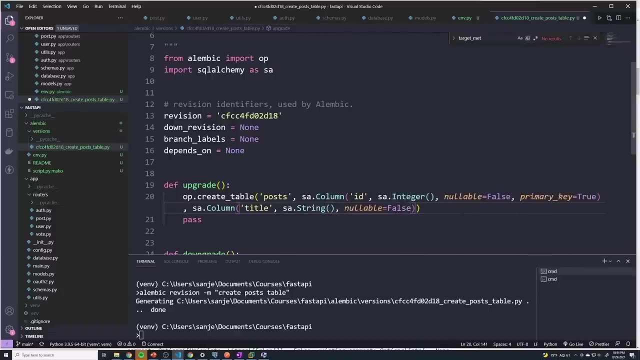 And so this is just going to follow the same exact pattern: sa dot column, And then this one will be the title. It's going to be a type of essay dot string, And this is going to be nullable equals false, And I'm just going to stop it right here. So we're going to just create two columns. 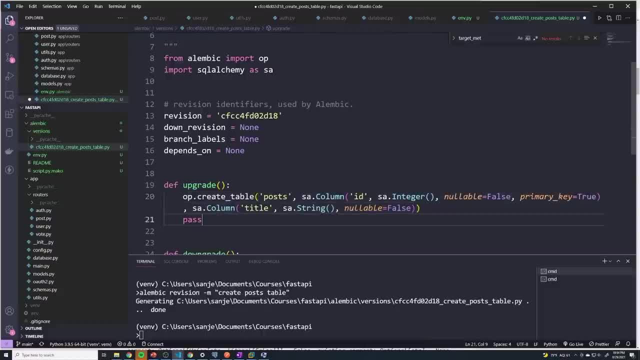 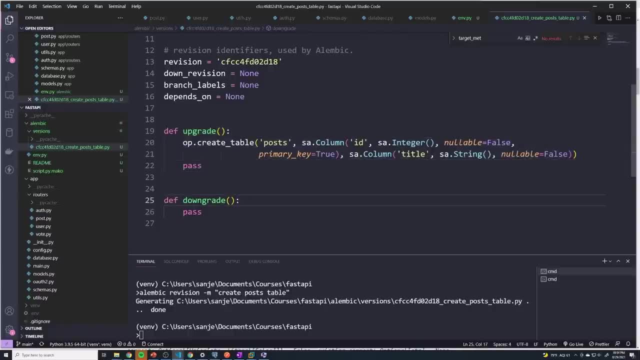 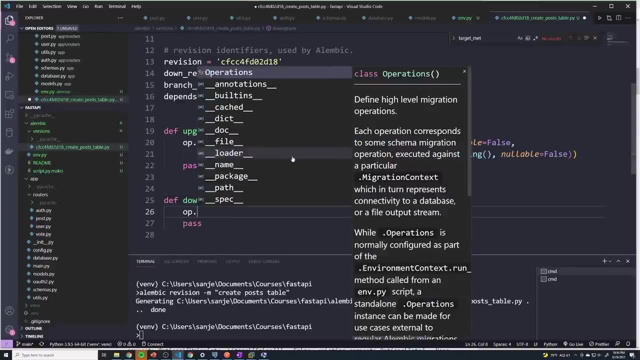 I don't feel like creating all of the columns that we had for posts, And so the upgrade function is done. However, we also have to provide the logic for undoing these changes. So if we create a table, what's the? how do we undo that? Well, we delete the table. So we do op dot drop underscore. 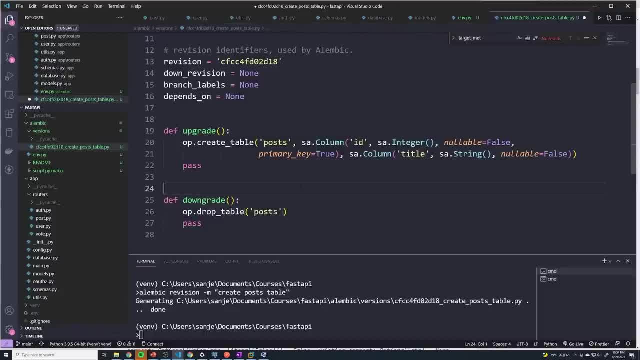 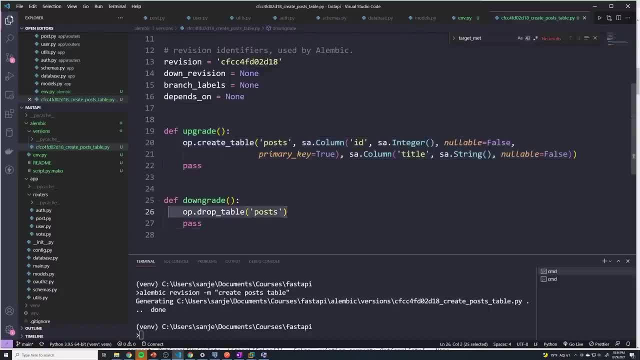 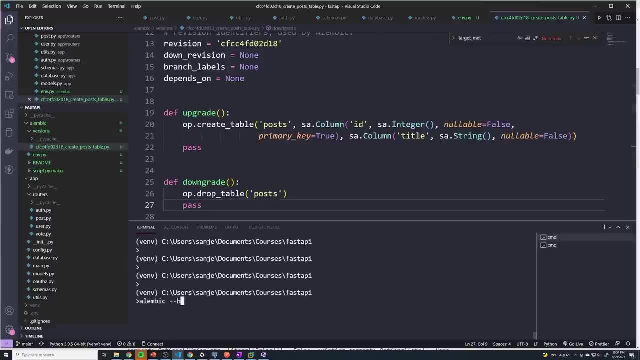 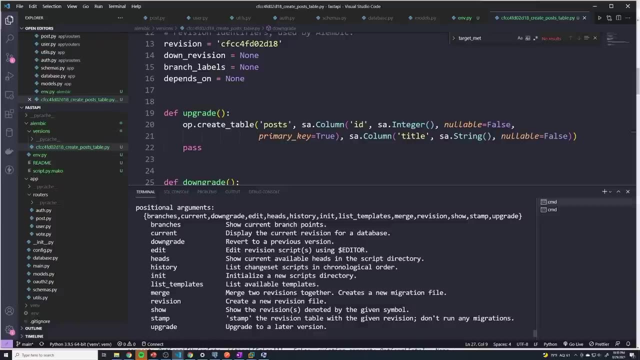 we should be able to make these changes And then we can roll back because we put the logic in for downgrading. So how exactly do we make these changes? Well, let's go to alembic, dash, dash, help, And let's see what commands we have. So we've got a couple branches. that's probably not it. 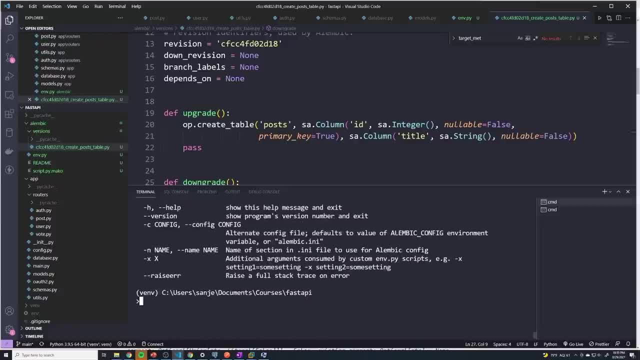 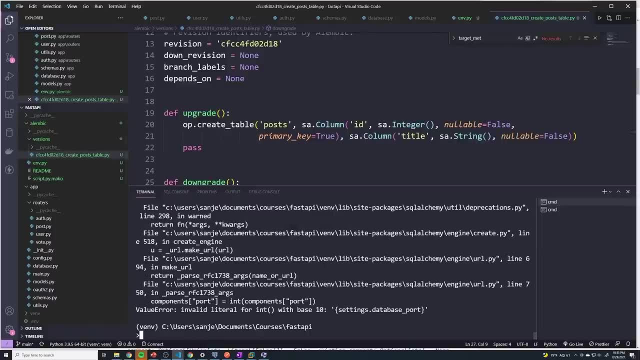 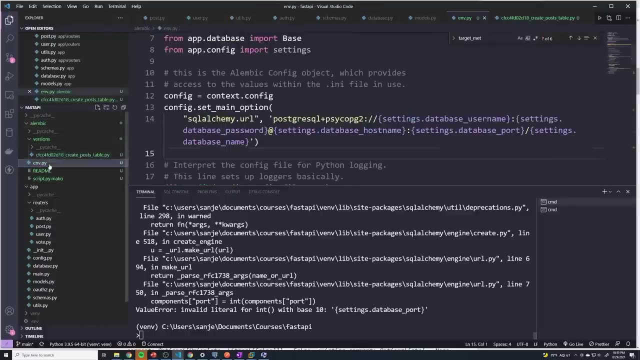 current. that's going to show us what's the current revision like, what version are we on, And if you actually want to see that, we'll see alembic current. Let me go back to my en V dot p? y file, And I made a very silly mistake. This should be an F string, So it wasn't actually doing anything. That's why it was kind of highlighted weird. So let's try this now again, we're going to do alembic current And it's not going to actually really give us any useful information at the moment because we haven't run any migrations right. we're kind of starting from a clean slate. So what we're going to do is we're going to go to these options. So let's go to these options And I'm gonna go to this one. let's go to the. 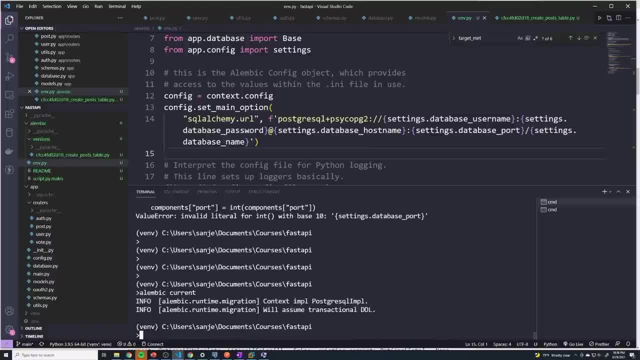 now again, we're going to do alembic current And it's not going to actually really give us any useful information at the moment because we haven't run any migrations right. We're kind of starting from a clean slate. So let's go back And let's just do a dash, dash help and see what. 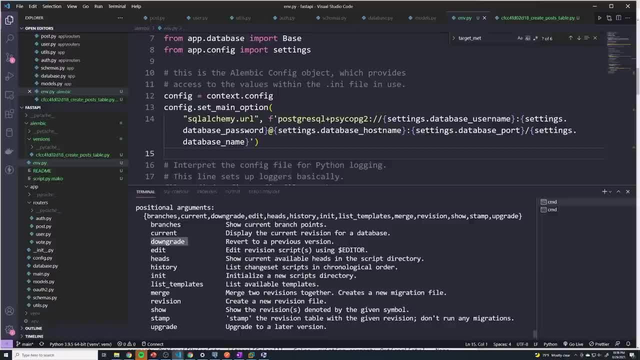 else we've got, So we've got a downgrade. well, we don't want to downgrade. edit, not really. Uh, heads, we'll come back to that history. Um, that's not gonna be useful because we haven't. 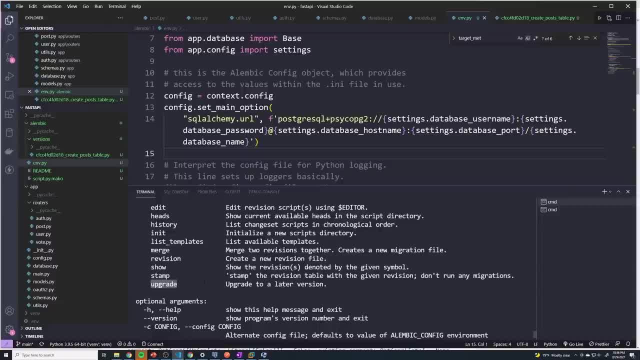 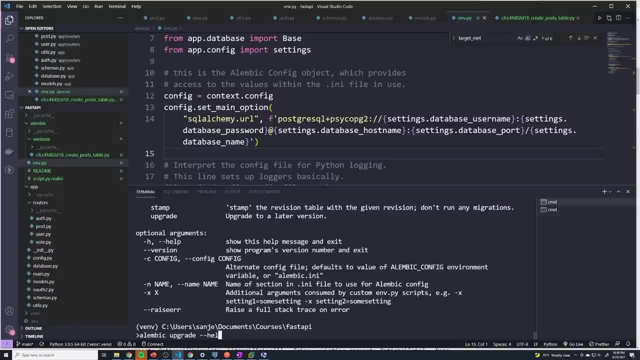 done anything. But if we go down, we want to get to upgrade. So this is what's important. So if we do alembic upgrade, we can just do dash, dash, help and we'll see what options we have. And so we have. 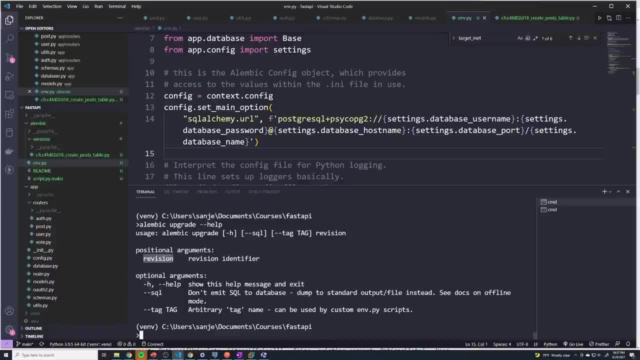 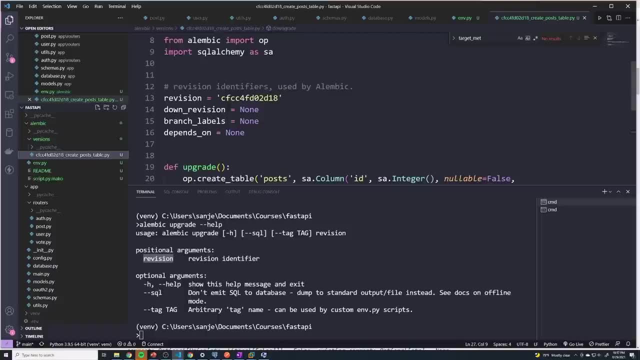 to provide a revision number to tell alembic like, hey, what version of our database do we want to go to? And so if you actually take a look at this specific revision, it provides a revision number. so if we actually want to get up to this point where it runs this upgrade, we provide these. 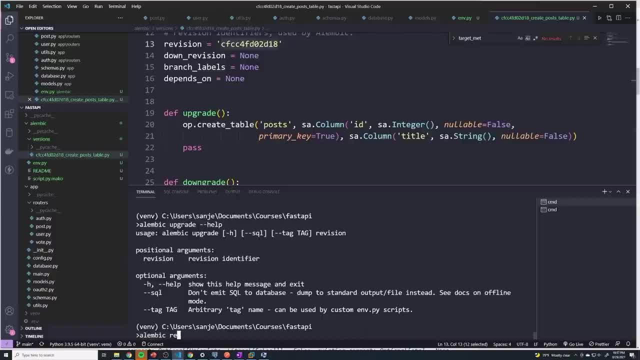 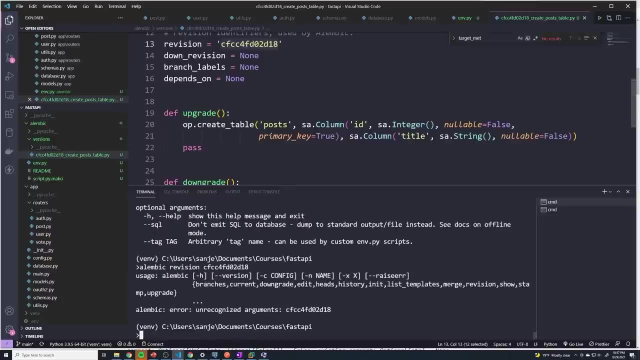 revision number So I can say alembic revision And then paste that. So let's run this and see what happens. Sorry, not, I didn't mean to type revision. I meant alembic upgrade And then that, not yet. 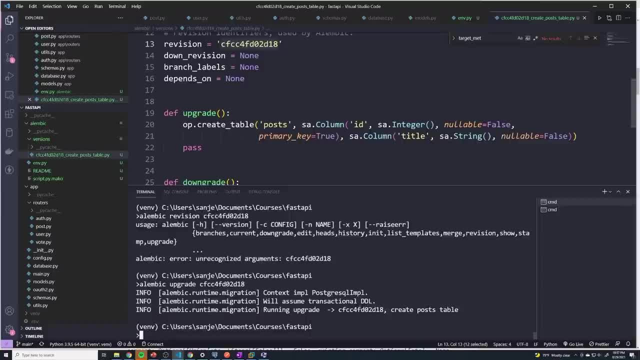 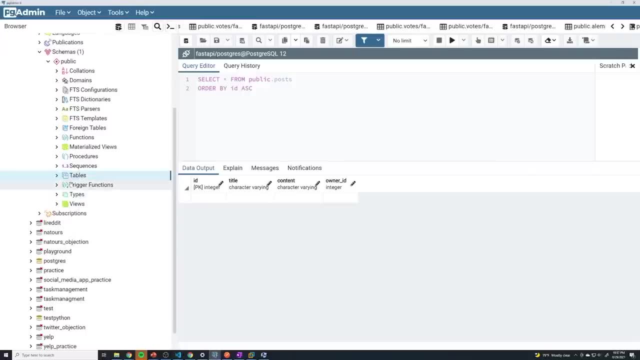 alembic revision. So that's going to upgrade it And so you can see it did a couple things says running upgrade and it said it created post table. So let's go to Postgres And let's just refresh this And let's see if it actually did something Right, And it looks like it created two tables. So 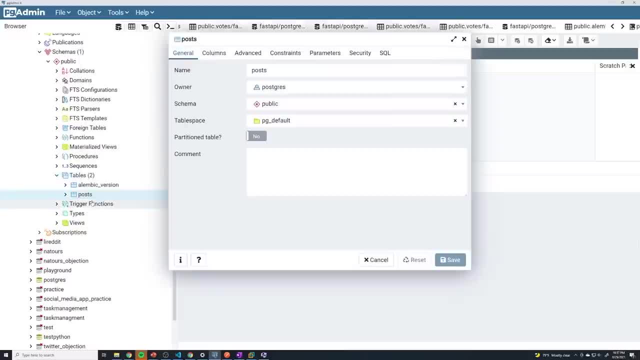 that's interesting. So we are. we see our post table And let's just quickly inspect this. We'll go to columns. you can see that it created these columns And this one got set to the primary key and both are not now, so it looks like it did everything it was supposed to do. But what is this? 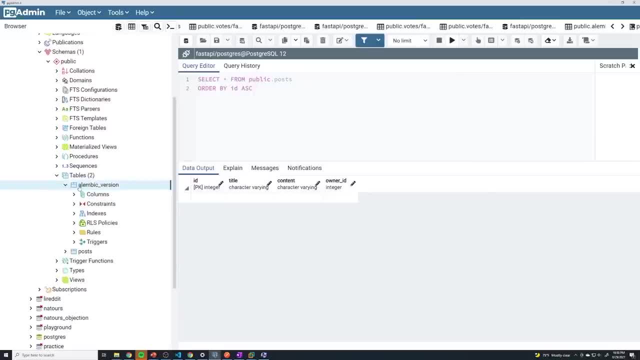 alembic versions table. Well, this is a. this is what alembic uses to kind of keep track of all the revisions, And so if we just go to view edit data, all rows, you can see that it just has one column at the moment which has the revision number. you can see it's. 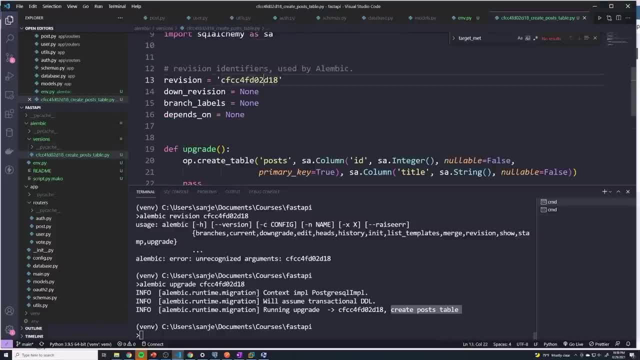 D 18.. And that's going to match up with this file D 18.. So that's all that's doing. So it will create a table for you automatically So it can keep track of all of the revisions, But make sure you. 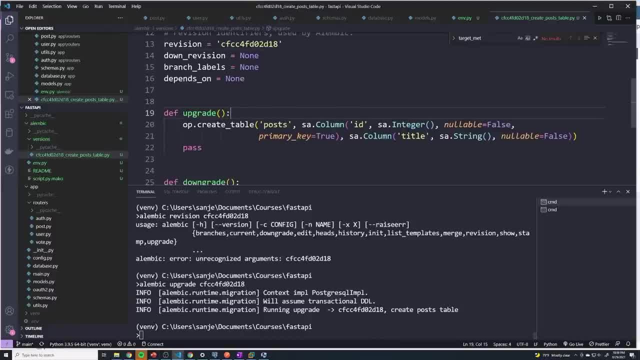 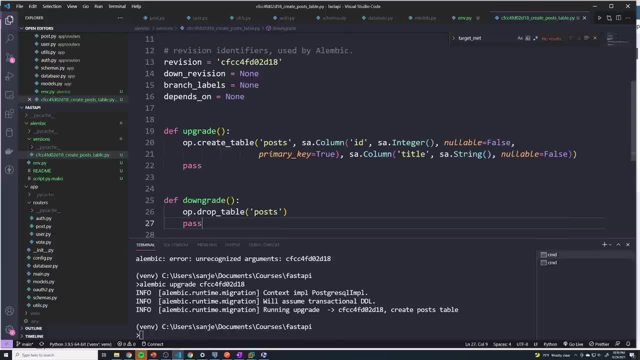 don't delete that, Okay, so that's cool. We just got our first table created through alembic And I think at this point you probably still don't understand the brilliance of a database migration tool. And that's okay, because we haven't really done much. 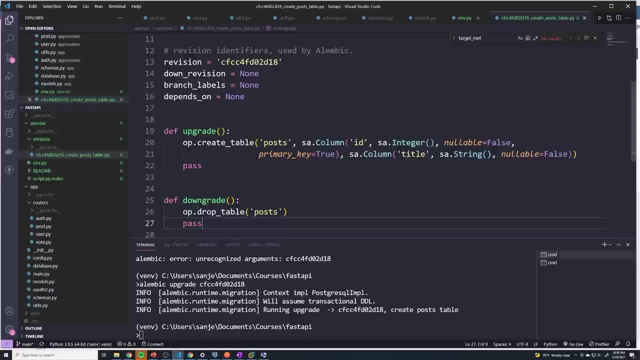 with it yet. So let's say that you know, as we're coding out our application, we realize we want to add a new column to our database, sorry, well, to our, specifically to our- post table. Well, we can create a brand new revision to add a new column. So let's say: if you take a look at our models. 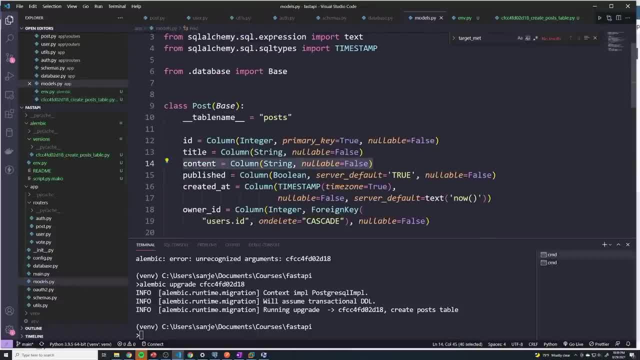 you know we have a couple other fields that are missing. So let's say we want to add the content column. Now I can type in alembic revision. So this is going to create a brand new revision. we'll give it a name and I'll say add. 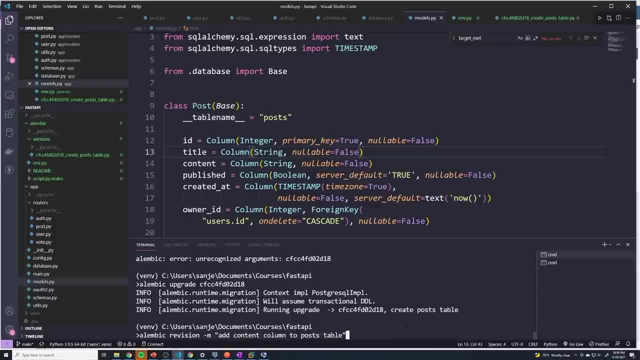 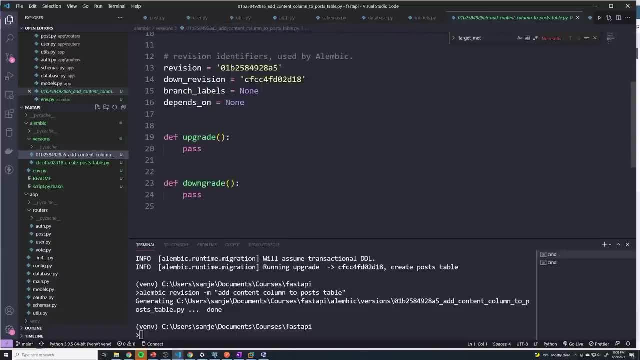 content column to post table. All right, and it's gonna create a brand new revision for us. And once again, we have to put in the logic for upgrading and downgrading And you can see that when we, now that we have more than one revision, we can see that there's also a down revision. So 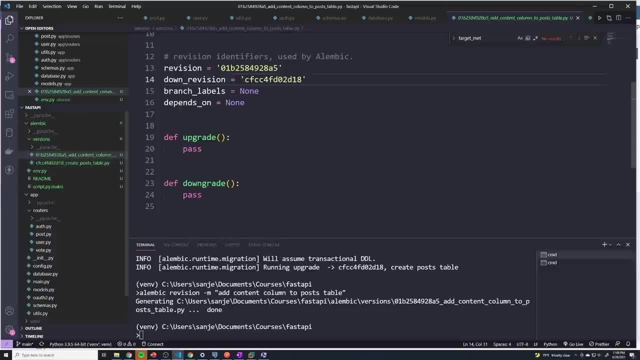 if you want to go down a step, it's going to go to the revision of the previous one. So let's put it in the logic for creating or adding any brand new column for content. And the way we add a new column to post table is we do op dot, add underscore column And then we specify the table we want to. 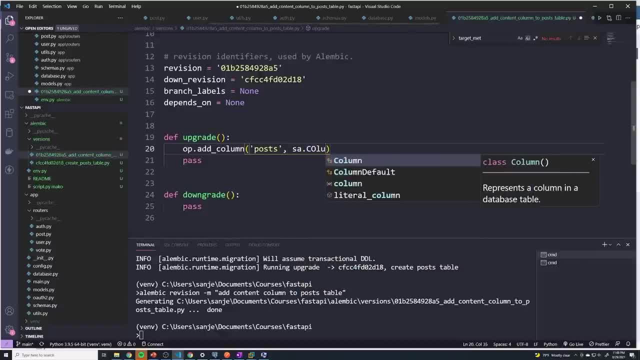 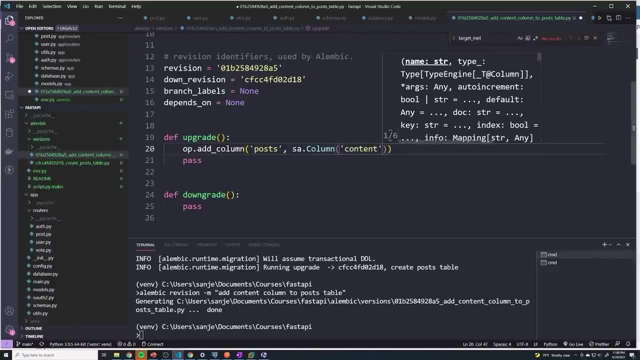 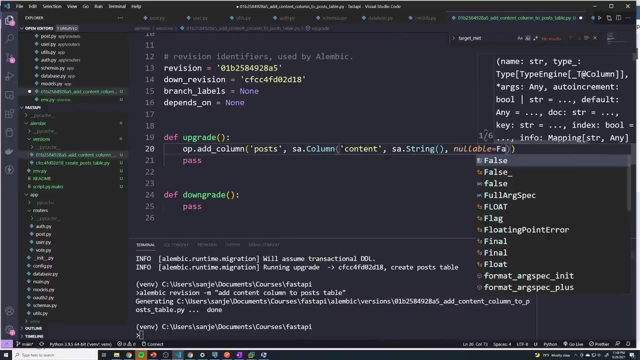 modify. So it's gonna be the post table And then we do SA dot column to define this column. So what's the column name? it's going to be content And there's gonna be a type of string And we're going to make sure that it's nullable, is set to false. 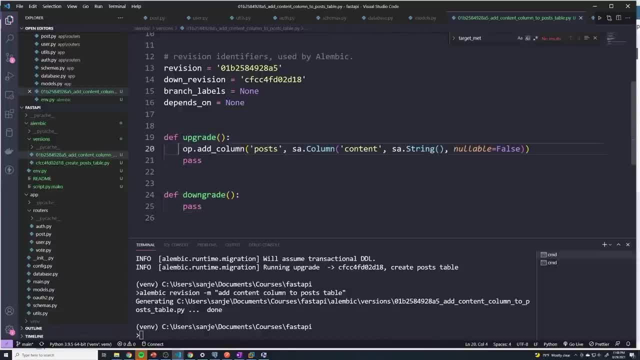 set up the upgrade function. you have to set up the downgrade function. So if we add a column, what's? how do we undo that? Well, we drop the column. So it's just op, dot, drop, underscore column And then from the post we have to provide the table that we want to drop the column from. 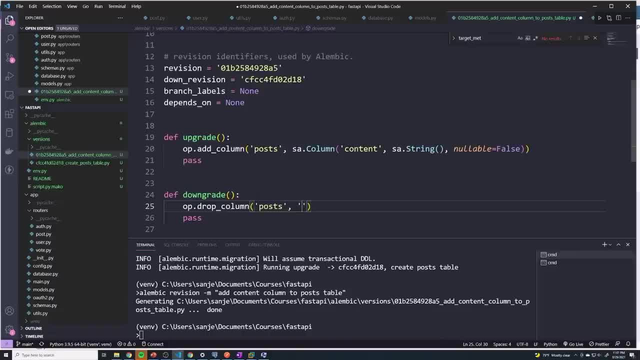 which is the post table, And then we need to provide the actual column we want to drop, which is going to be content. So we'll do content, Okay, and so let's test this out. First of all, we'll run a few new commands. So alembic. 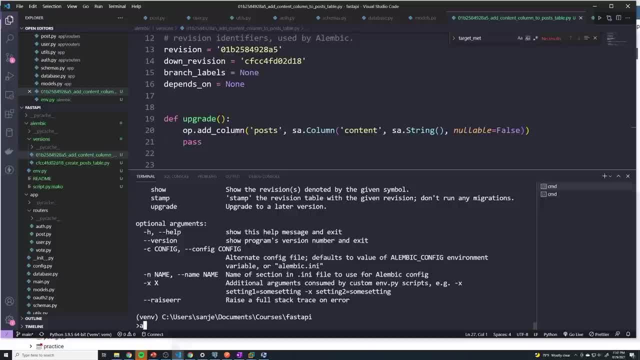 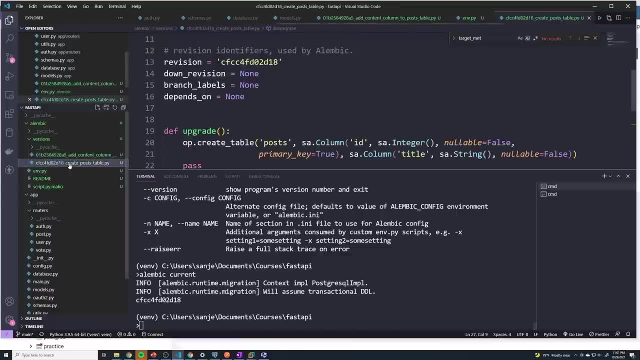 All right, and let's see what the current revision is. So if I do alembic current right, we can see that we are currently on 2d 18.. That's the revision. So this is the the revision where we created the post table. And if I type in the alembic heads: 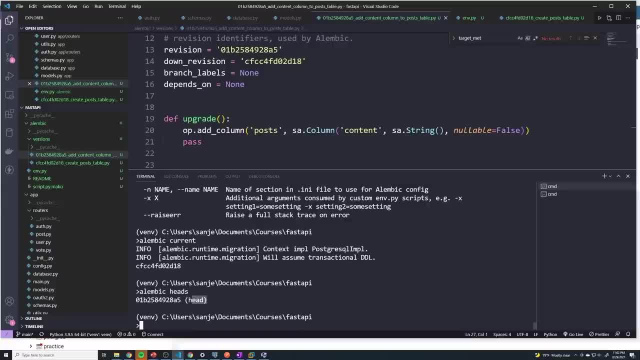 we can see that the latest revision is actually 298, 298 a five, which is that new one we just created. So if we ever want to get to the latest revision, that's what's referred to as the head. So I can say if we want to. 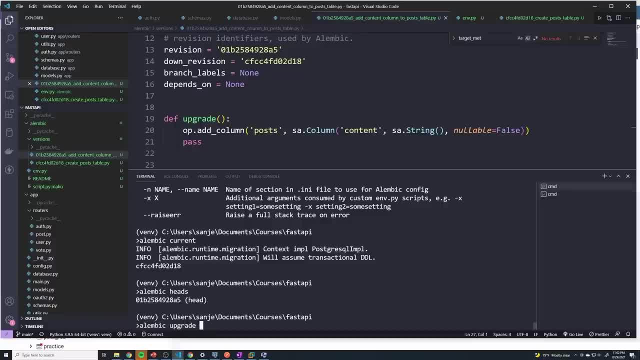 you know, upgrade to that revision. I can say alembic upgrade, like we did before, And I can grab the revision number like this. Or, because it's also happens to be the head, I can just say alembic upgrade, head, and it's gonna do the same thing. So let's try this. 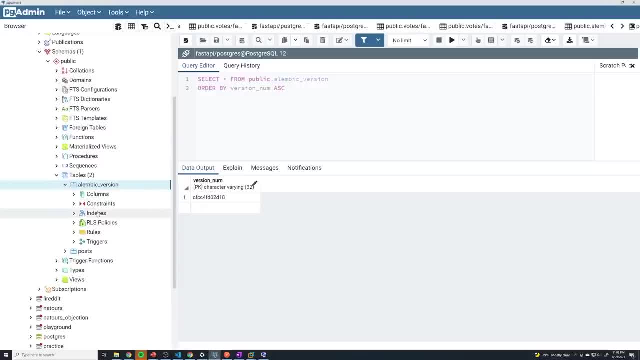 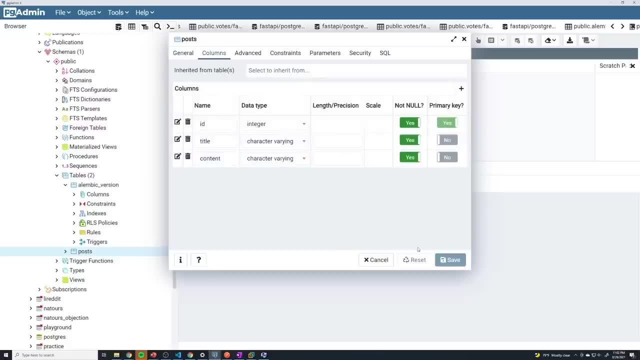 All right, it said it added a content column. we'll go and check this in Postgres- And I'm just going to refresh this table- And we'll go into properties And we can see that we added the content. Now Let's say that after working on this for a bit, 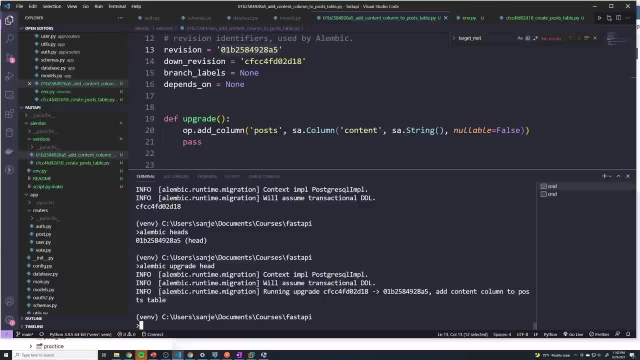 we realize we want to undo these changes, for whatever reason. maybe we no longer want the content column. So how do we actually roll back? Well, the, since upgrading makes the changes, we're going to do the opposite. So we can do alembic downgrade And then, if you want to, just 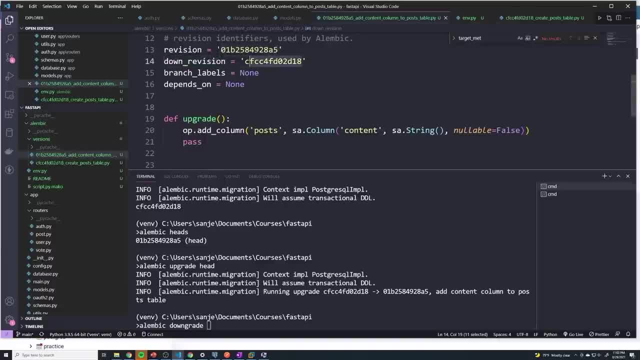 roll back this revision. we can see what the down revision is. So we can just say this and just paste that in there. But we can also do a few other things. we can also say minus one. So when I say minus one, that means I'm going to go back to one revision earlier. 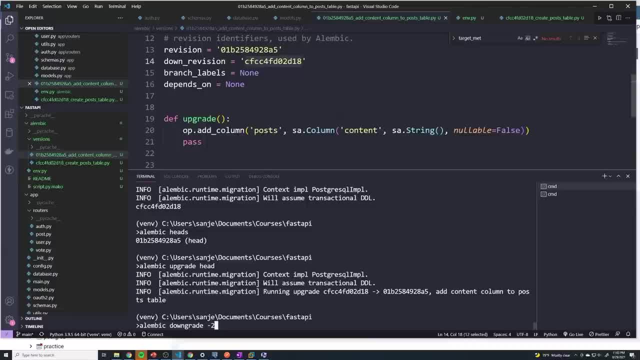 And we can even go as far back as we want. So if I say I want to go back to minus two, it's going to go back to two, But we just have one. So I'm just going to say minus one or I can just paste in: 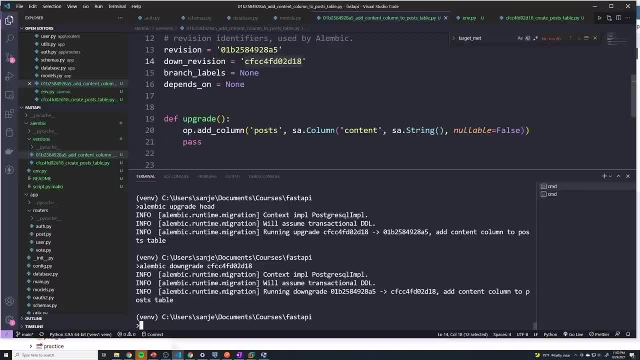 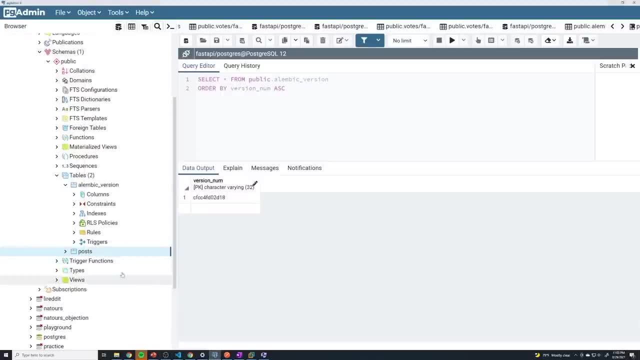 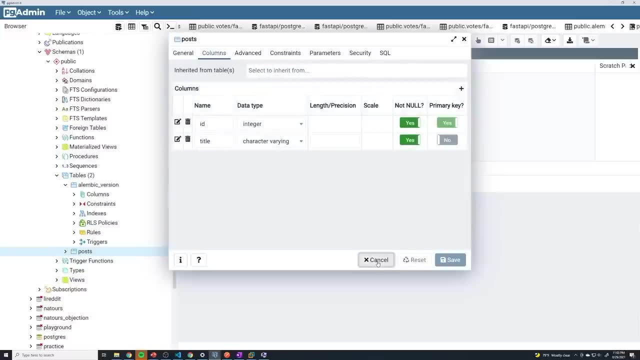 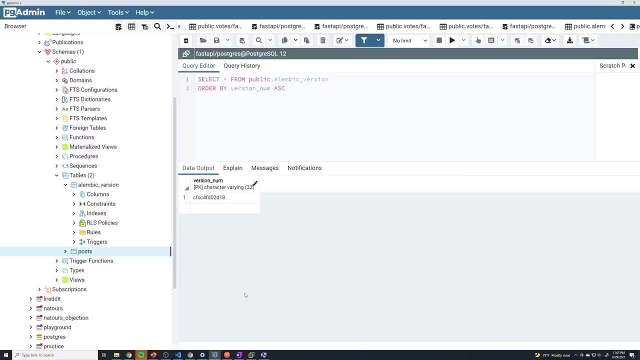 the revision number And so if I run the downgrade, you can see that it ran this downgrade. And if I go and refresh this and then go to properties columns, we can see that we no longer have a content column. And that's how easy it is to downgrade or roll back your database using a database. 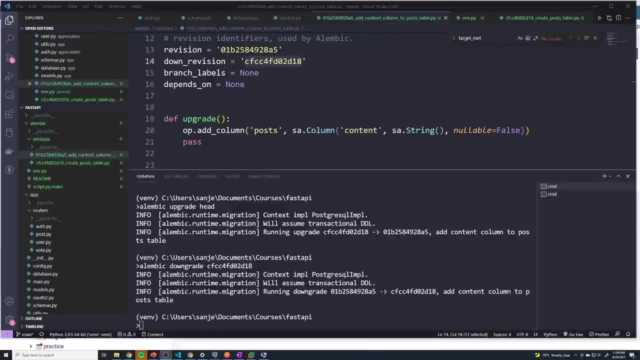 migration tool like Alembic. Okay, so we got our post table. we're not going to worry too much about that. The next part of our application was: hey, let's implement a user functionality, let's make it so that users can sign up and log in. So now we need to create a user's table. 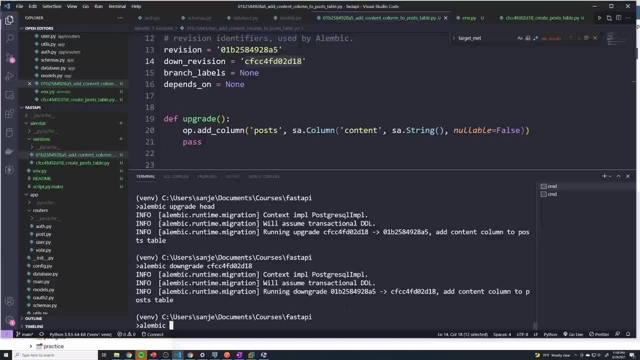 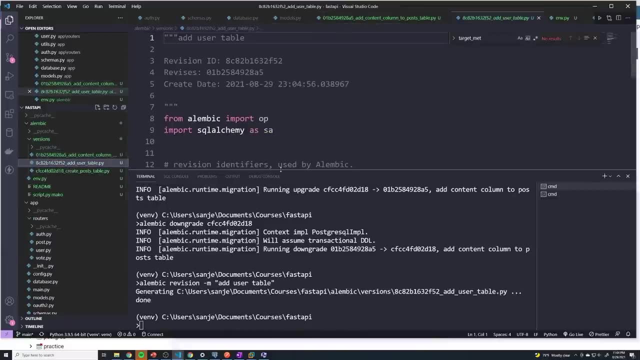 How do we do that? Well, let's set up a new revision. we'll do Alembic revision, dash M, And I'll say add user table. All right, so we've got our brand new revision And we have to set up the upgrade and the downgrade. 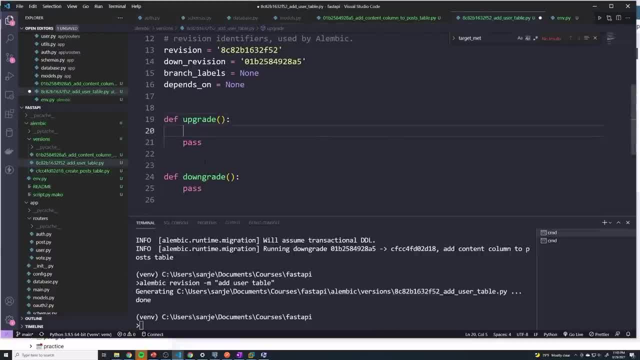 Now for this. I don't want to just type this out, you know, one by one. it would be kind of slow and boring for you guys. So I've, actually I'm just going to copy and paste this from my notes And. 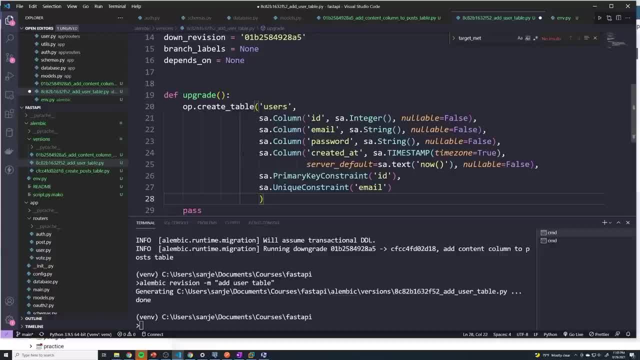 if you want to follow along, just you know, pause the video and just write this out, But we'll just quickly, you know, walk through exactly what's happening. So, once again, we're using the create table method. we're going to create a table called. 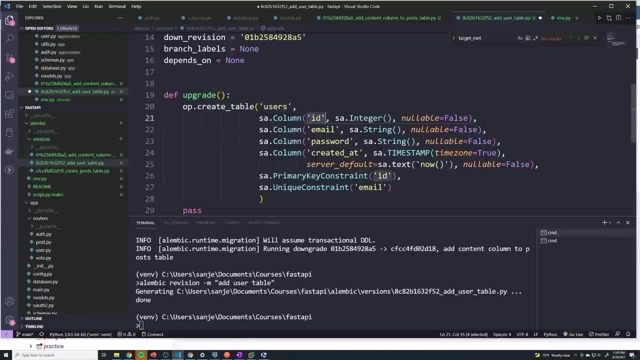 users. And then we're going to set up all of our columns. So we've got a column called ID, which is an integer set to nullable equals false. you notice how I haven't set this to be the primary key here. That's because there's two different ways to set the primary key, You know. 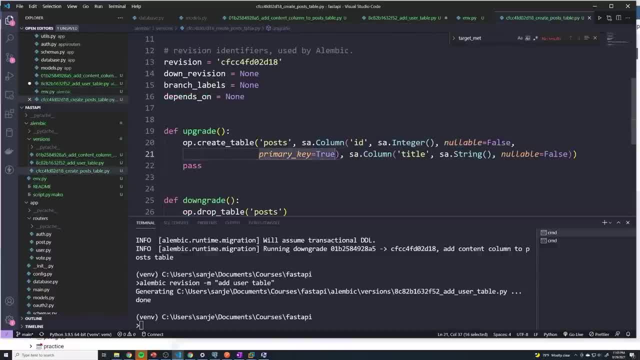 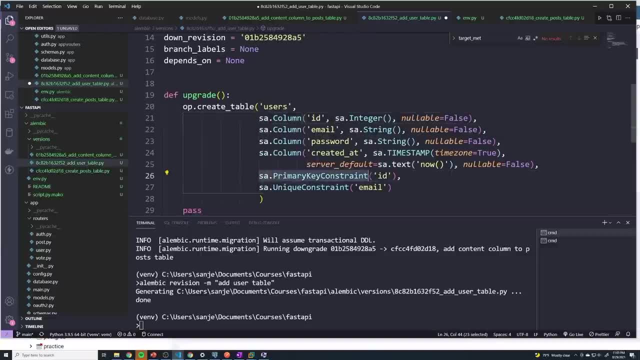 if we go back to the previous one, we set this to be primary key equals, true, But on this one, if you actually go all the way down to the bottom, you can see that we can add in a constraint as a primary key constraint, And then we pass the name of the column. that's going to be the. 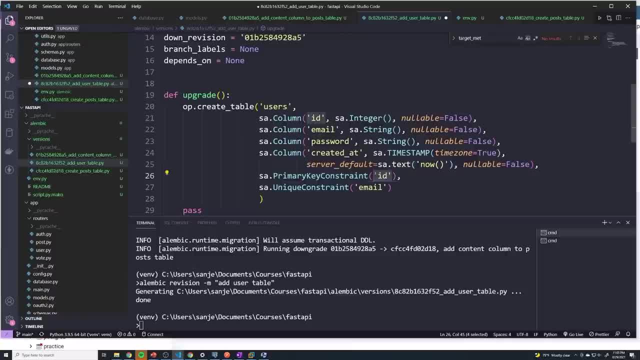 primary key, So they both do the same thing. It's just whatever method you prefer. Now we've got the email column, which is going to be set to nullable, equals false, same thing with password. then we've got the created at, And so here it's going to be a type timestamp And you'll see that. 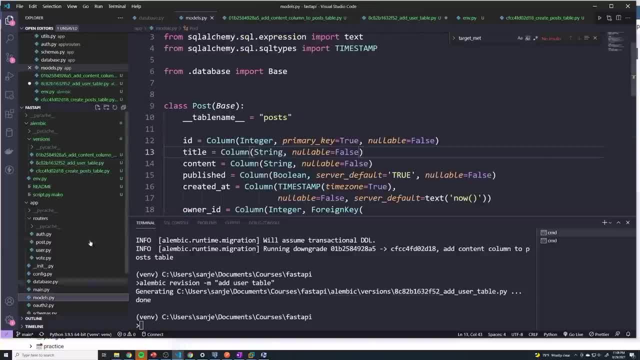 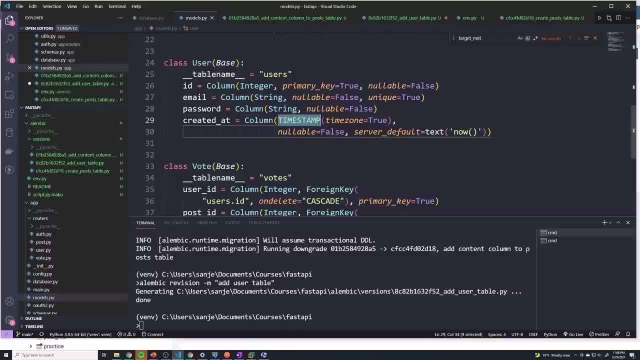 this is all coming from SQL alchemy, essentially Because if we go to our models and we go to our user table, it's the same thing. type timestamp, timezone equals true, nullable equals false. server default equals text. Well, that's created that, but yeah. 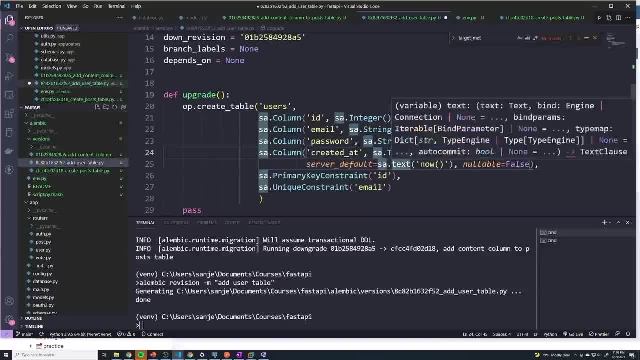 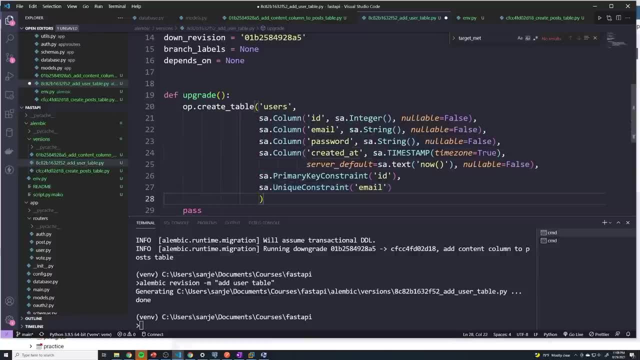 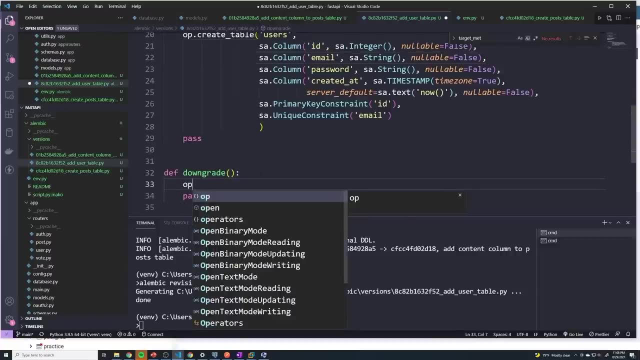 Doing the same thing, So server default. and then we grab sa dot text: now nullable equals false. And then you can see that we added a unique constraint under the email field to ensure that we can't have duplicate emails. And then to downgrade we just do op dot drop underscore table. 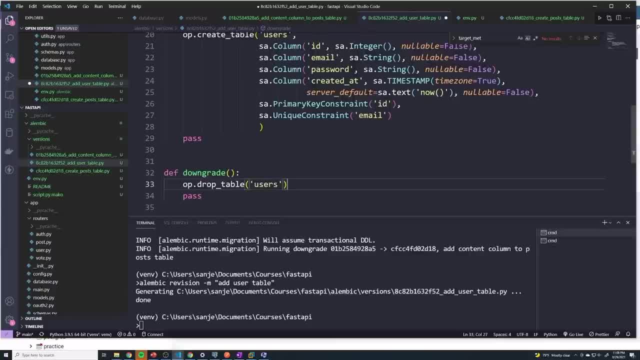 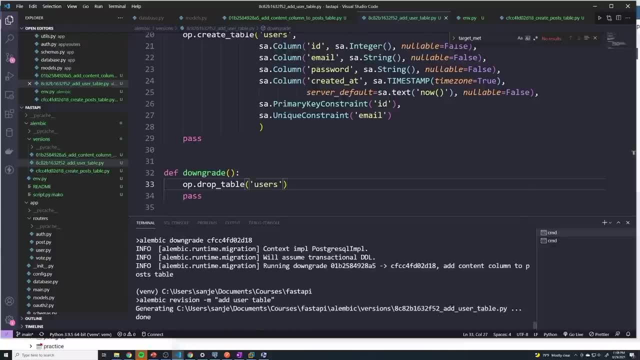 users, All right. And so, once again, if you want to see where we currently are, because we're going to be doing the same thing, we're going to be doing the same thing, So server default. and then we grab sa dot text now nullable equals false, And then you can see that we added a unique. 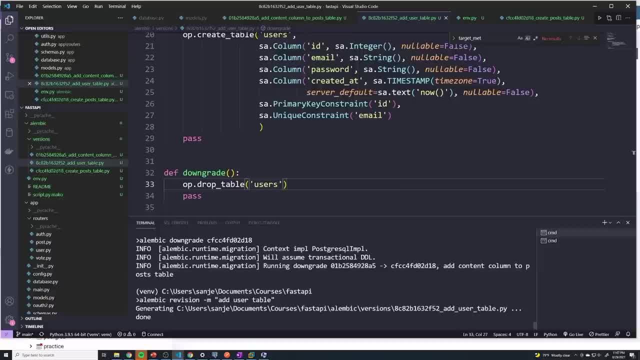 constraint under the email field, So server default. and then we grab sa dot text: now nullable equals false. And then you can see that we added a unique constraint under the email field. Remember we had originally upgraded, added the content column, but then we downgraded, So where? 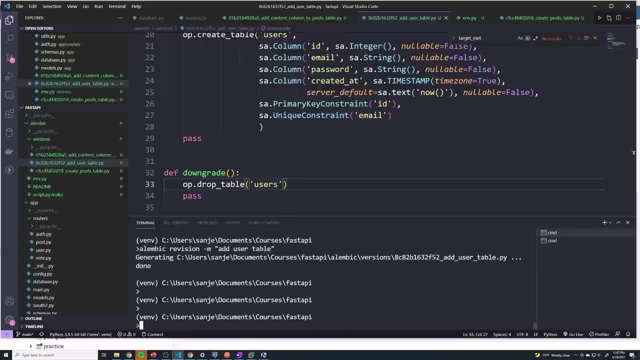 exactly are we from a revision perspective? Well, let's do alembic current. You can see that we're on 2d 18.. So we're back on that first revision And we can also do an alembic, I believe it's. 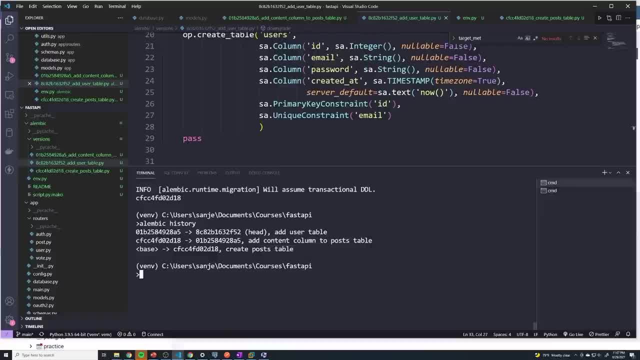 history And you can see the history of our revision. So we created post, add content column to posts and then add user table And this is the head. So if you want to go all the way to the front, to the latest, you would just do alembic: upgrade head. 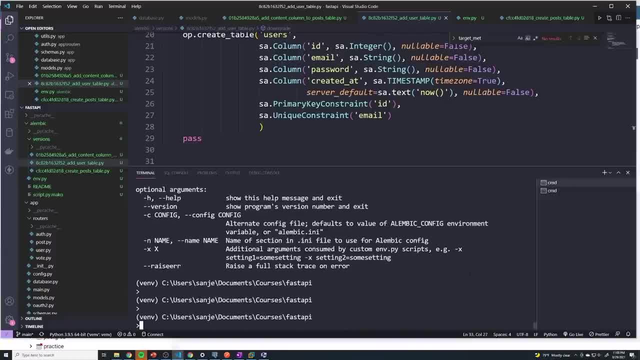 And I think there's one more I want to show you. Yeah, that's okay. So we're going to do an alembic And let's say that we just want to go and go up one revision. So adding one revision is going to add that column back. we can do alembic. 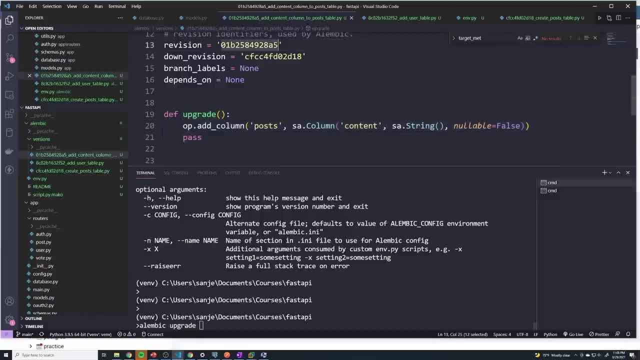 upgrade And we can either put in the name of this revision Or we can upgrade one level. If we want to go all the way to the latest, which is going to be adding the user table, we can say head. we can also go up to revisions. So if I do plus two, that's going to. 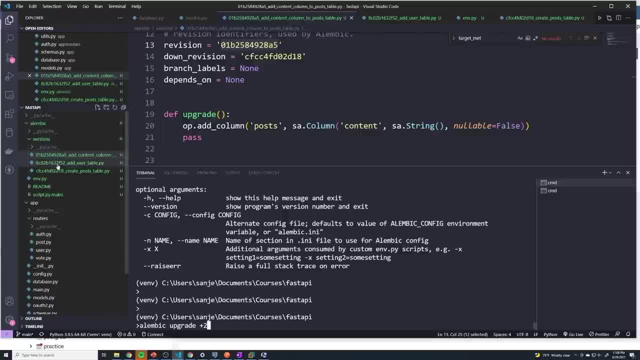 go up to add content column one. that's the first revision and then one more which is going to go up to the latest in this case. So there's a lot of different ways to get there. I'm just going to go to the latest. So this is going to add the column back in the post table and then add the users table. 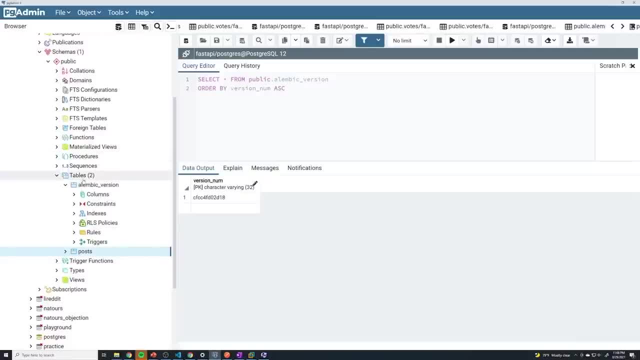 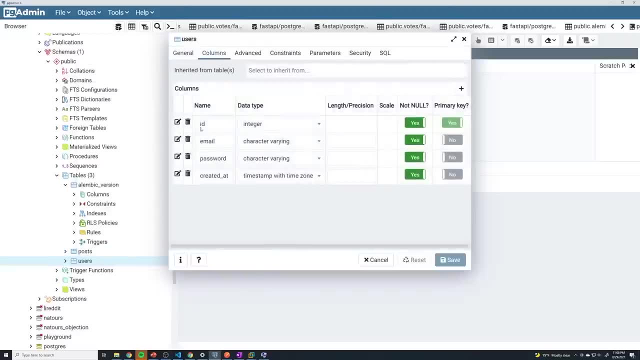 And you can see that it went ahead and added the users table. So, if I refresh this, we can now see that we have a users table And hopefully all of the properties are there. You can see all of these have been set. constraints: primary. 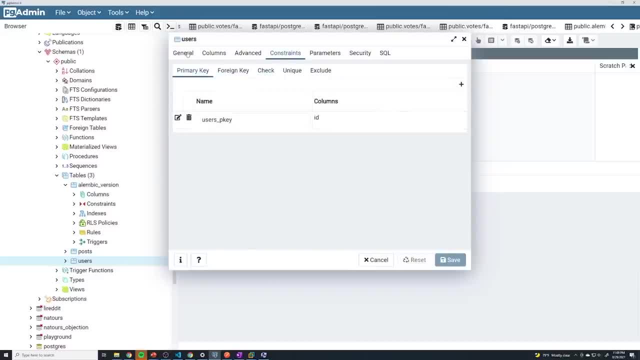 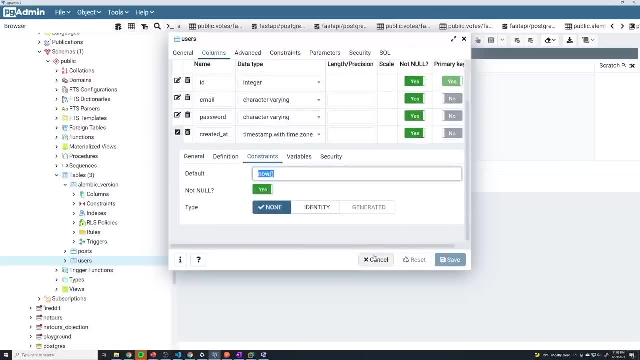 key is set And anything else. everything else looks good. I guess one thing just to check is the created at. So if we check the constraints here, you can see that we're going to grab the current time. Perfect, All right. so after we had added the user functionality, 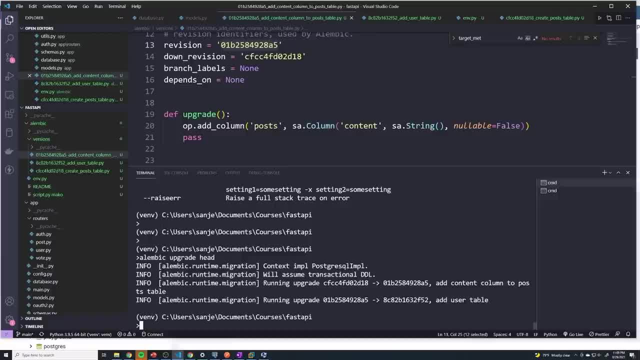 the next thing we had to do was we had to implement the relationships between users and posts. So we had to set up that foreign key that linked the user table to the post table or the post table to the user table. So once again, we're going to do an Alembic. 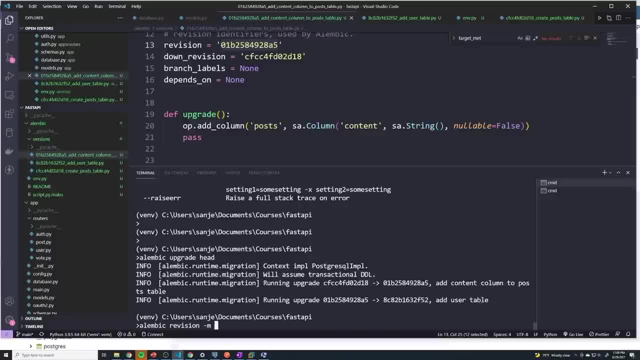 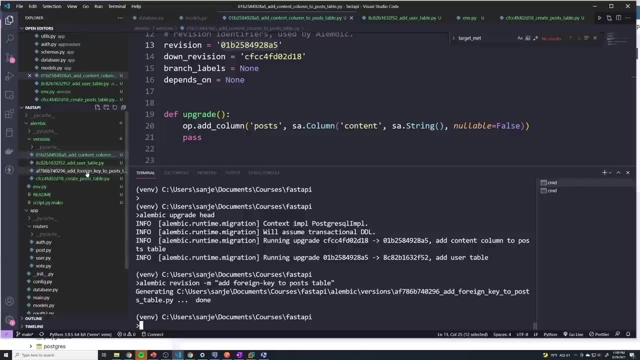 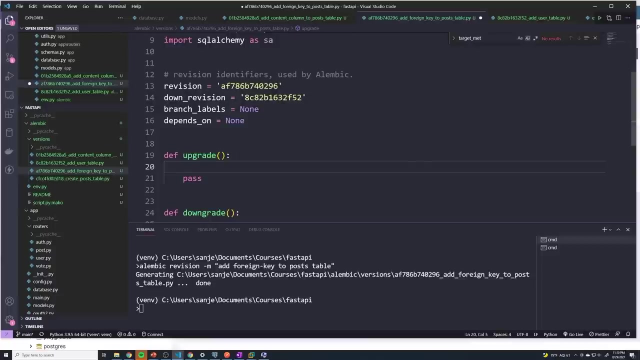 revision dash M. I'm just going to say: add foreign key to post table. All right, we got our new revision And what we're going to do is we're going to: first of all, we have to add a column to our post table called owner ID, And that's going to. 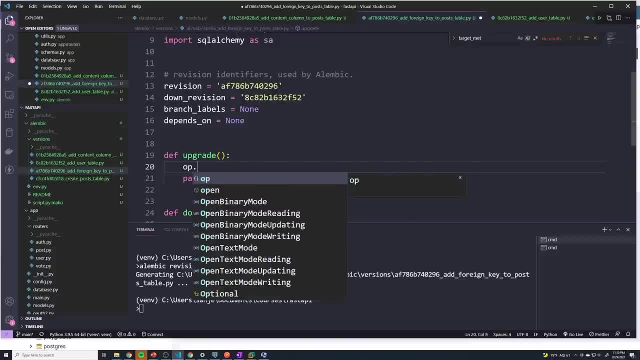 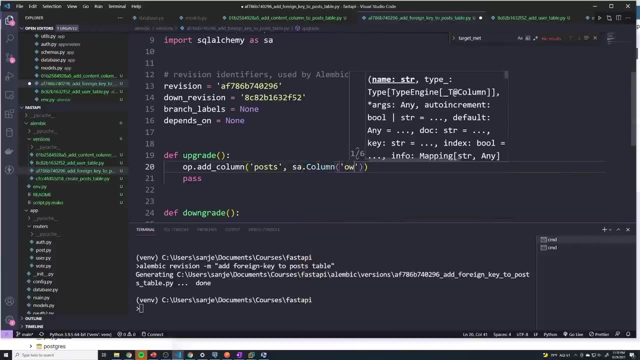 be the one that has the foreign key constraint. So we have to do op dot add column And we have to specify the table we want to add the column to, which is going to be the post table, And this is going to be sa dot column. We're going to call this owner underscore ID And. 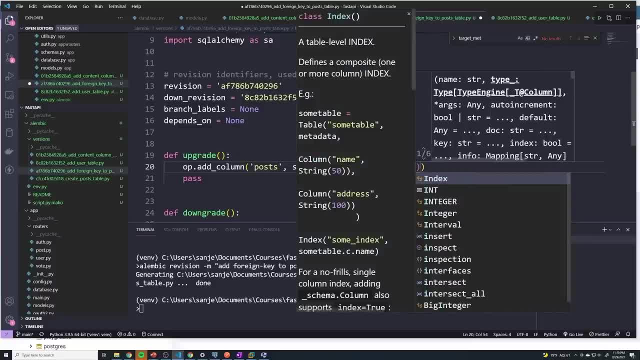 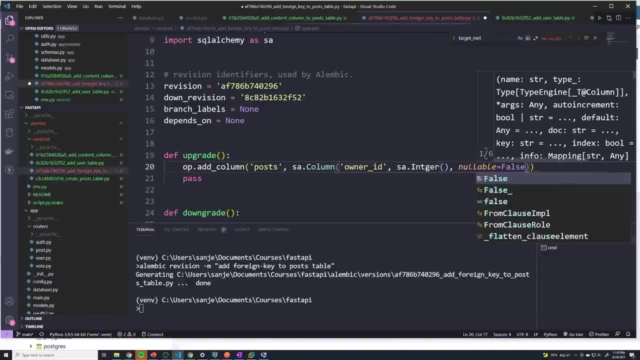 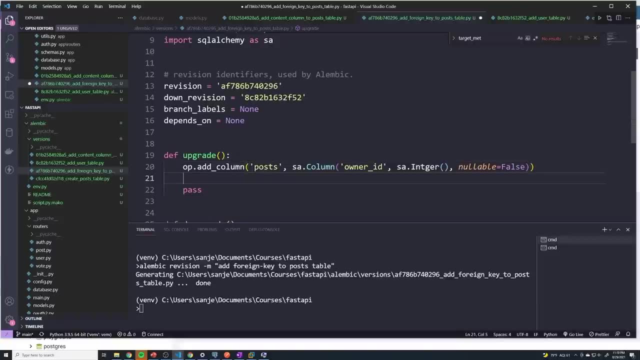 it's going to be a type of sa integer, And nullable is going to be set to false. Alright, so we've created the column. Now we have to set the link between the two tables, which is going to be the foreign key constraint, And so to do that is a little bit confusing. 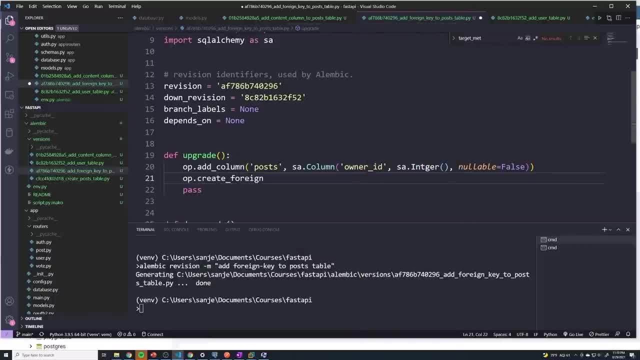 at first for me, because the documentation is a little bit hard to read sometimes. So you do create foreign key, Then you have to give it, you know, some arbitrary foreign key name. I'm going to call this. posts, underscore users. underscore FK. This is the foreign key between the posts and the users. 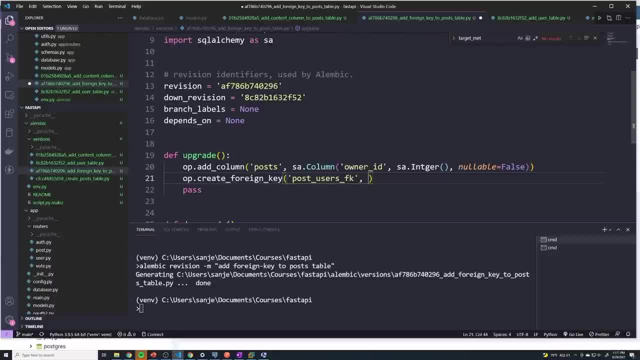 table. And then we have to specify what is the source table of the foreign key. So this is going to be the foreign key for the post table. So we're going to say source underscore table equals post. Then we have to reference the, the remote table, which they call a referent. 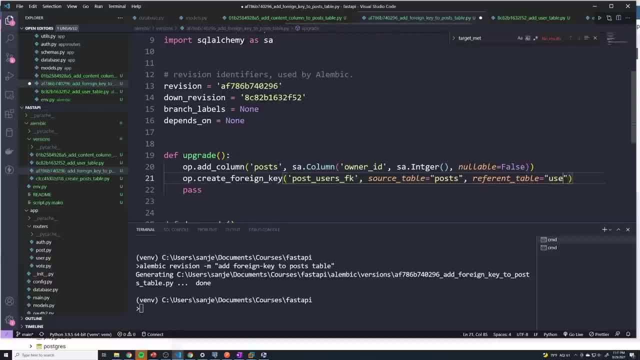 on, And so this is going to be the users table, And then we have to specify what is the local column that we're going to be using. So the column in the post table And that's going to be owner underscore ID, which is the table, the column that we just created, And then 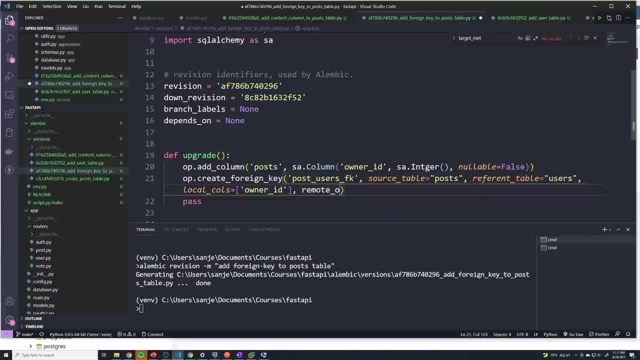 finally, we have to specify the remote column in the users table And this is going to be set And we're also going to set the on delete to be cascade. And yeah, by the way, the remote column is going to be the ID field of the user table. 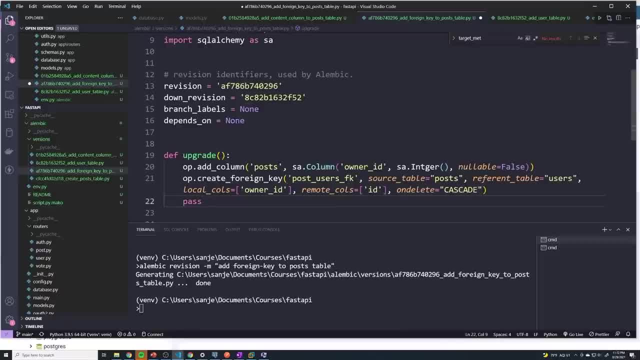 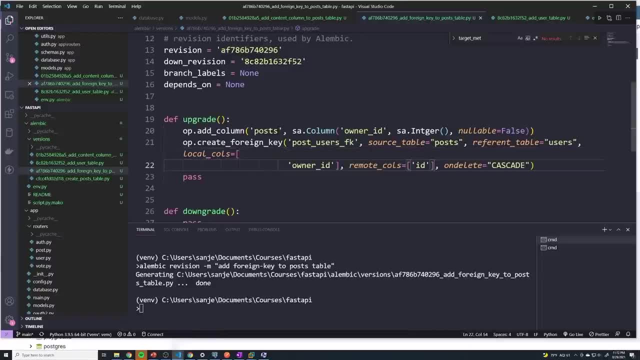 And we want to make sure we have the on delete as well, And that pretty much. Oh, what happened there? It's a weird way to format things. All right, well, it wants to format it that way, So I'm just going to leave it like that. 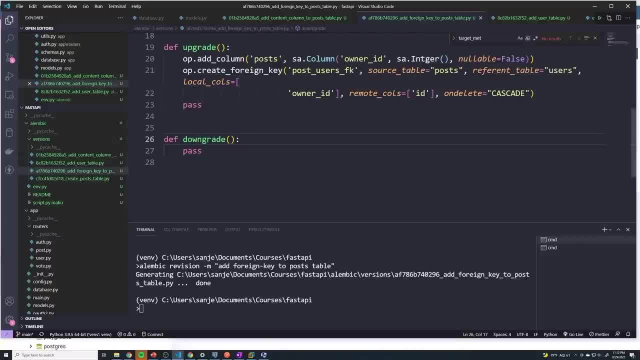 Okay, Let's set up the downgrade Now. So we have to undo those changes. We'll do op dot drop underscore constraint And then we just mentioned the name of the constraint, which is post users FK. We have to specify the table that we're removing it from. So it's on the post table. So we 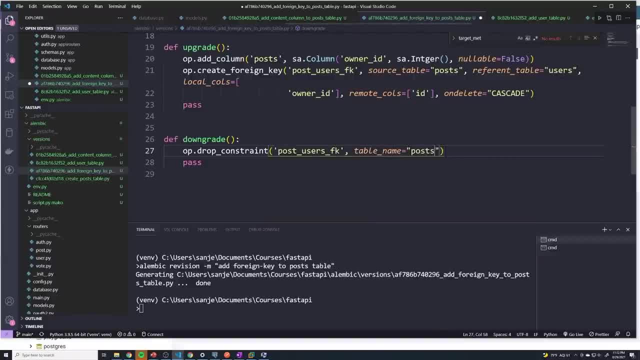 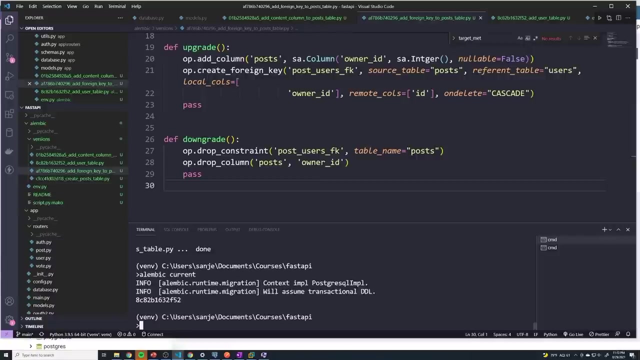 do table name equals posts, And then we have to drop the column, So we do op dot, drop score ID. And where does this column sit? It's in the post table And it's called owner underscore ID. All right, And so if I do an alembic current, we're on F five to an alembic heads. let's. 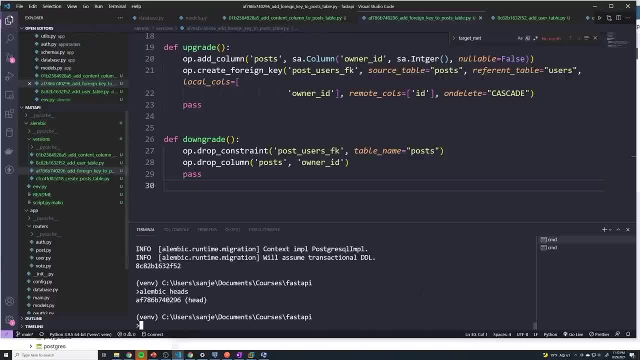 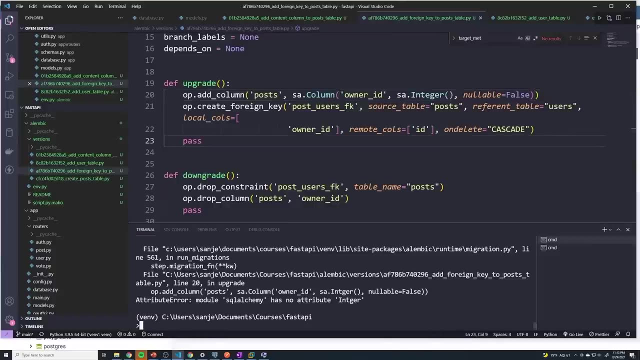 see what the latest one is. it should be 296, which is this one. So let's do an alembic upgrade head. go to the latest, And I have a typo, So this should be integer. All right, looks like it ran with no issues. Let's double check that the foreign key is. 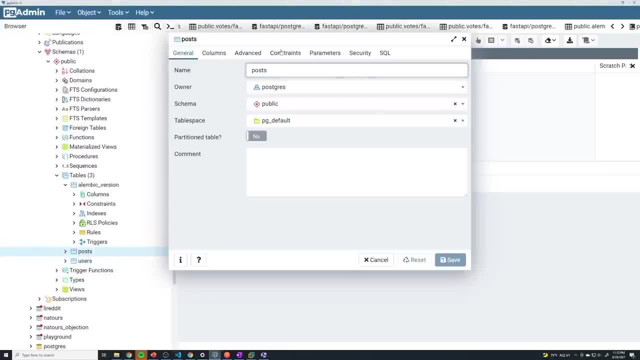 there. now, If we go to post properties, constraints, foreign key, you can see that we have our post user FK And we can see that it points from owner ID in the post table to ID in the users table And, if you want to, you can go under actions and see that cascade has been. 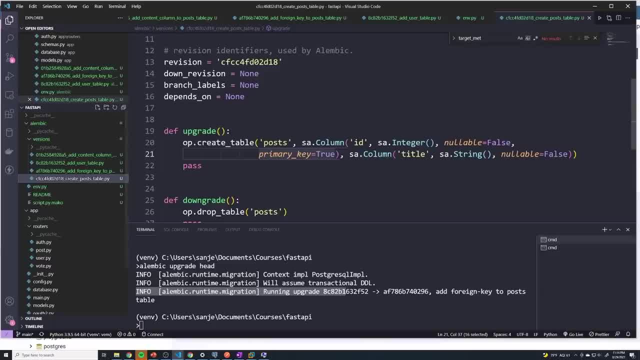 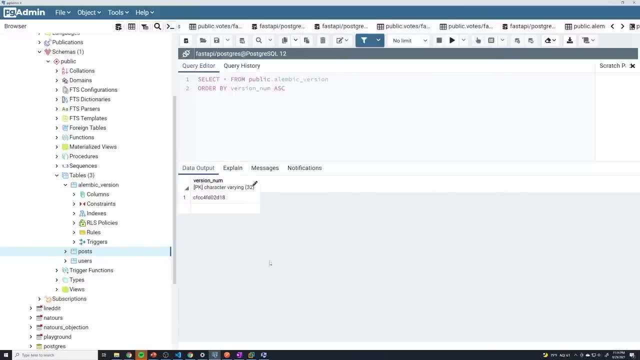 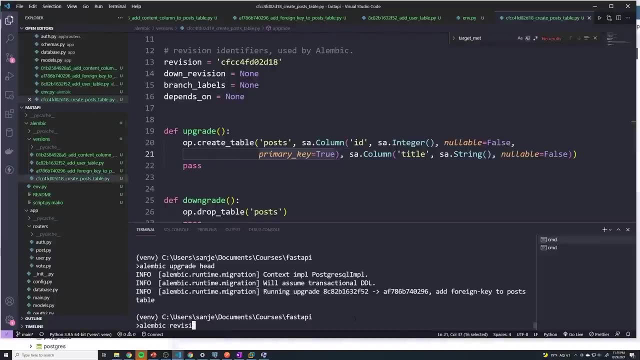 set to on delete. Now in our post table at the moment, you know, we didn't implement all of the columns that we actually have in our application. So I figured out why not just go in and add it might as well. So I'm going to create a new revision, All right, and then we go to 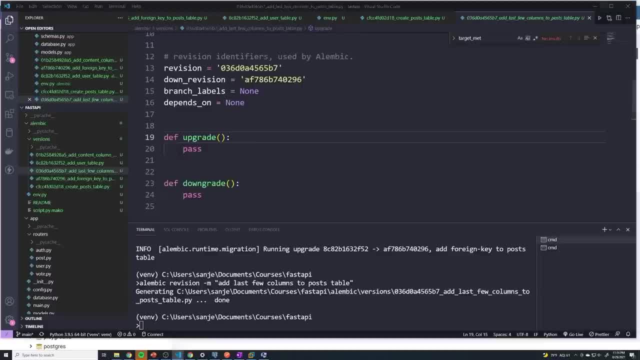 that revision. There's really only two more columns. There are columns that we have to add, And this is. I'm once again going to just copy and paste from my notes, just because I don't want to waste your guys time too much. But 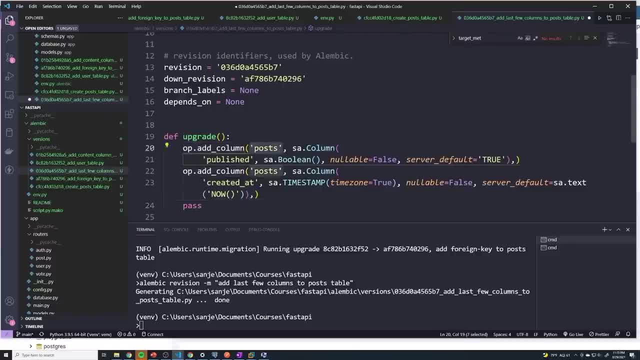 you can see, here we're going to do an add column And we're going to add it from our added to our post table. And then here we're going to specify the parameters of the column. So this is going to be called publish, it's going to be of type Boolean and nullable. 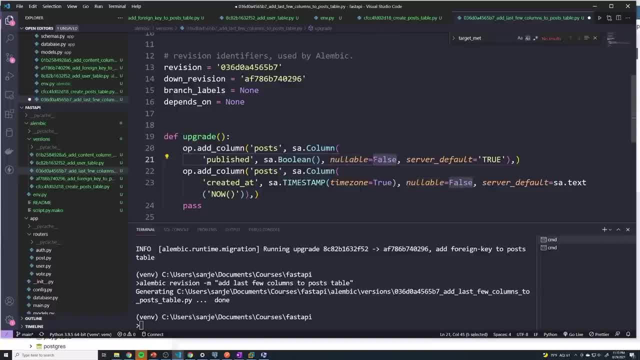 equals balls, And that's not correct. it should actually be nullable- equals true- Right. It should be Actually. no, it was false. It should be nullable equals true, And that's not correct. It should actually be. nullable- equals true- Right. It should be actually no. 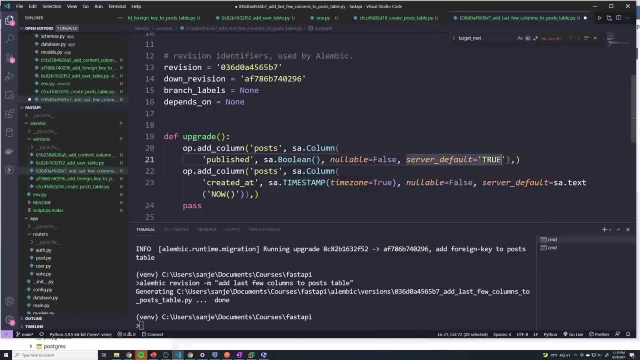 it was false. And then server default is set to be true. So if we don't provide it, it's going to assume it's true. And then the next one is the column for created at. So once again at the post table we're going to create a column called created, that it's. 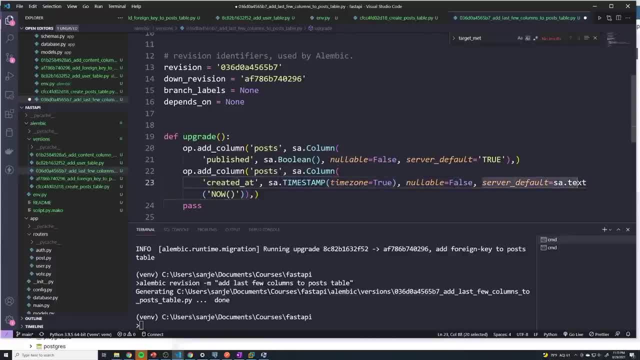 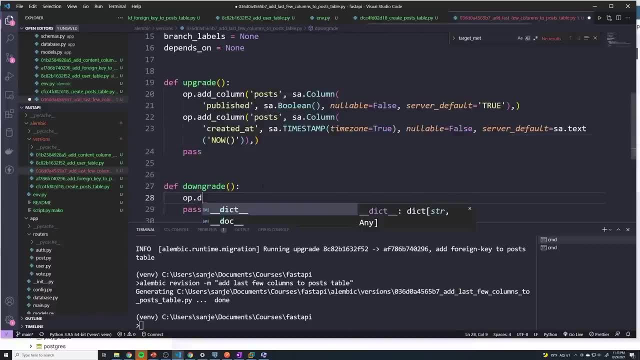 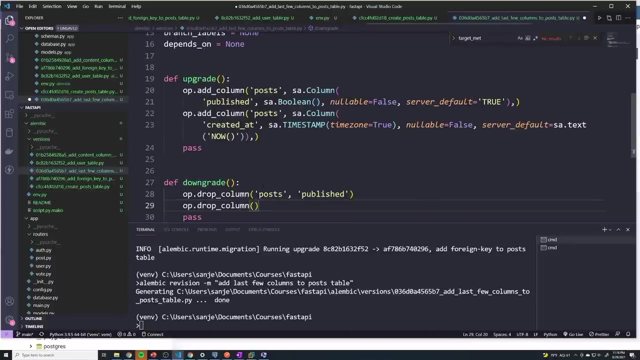 gonna be a type timestamp- nullable, false- and then the default means we're going to grab the current time And to downgrade. we're going to delete those columns, so we're going to do another block here and then around here we're gonna copy that GI. 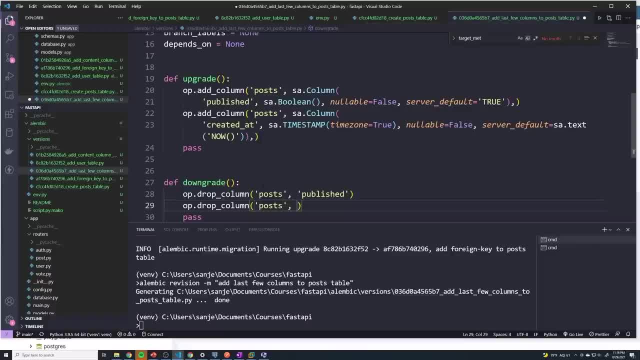 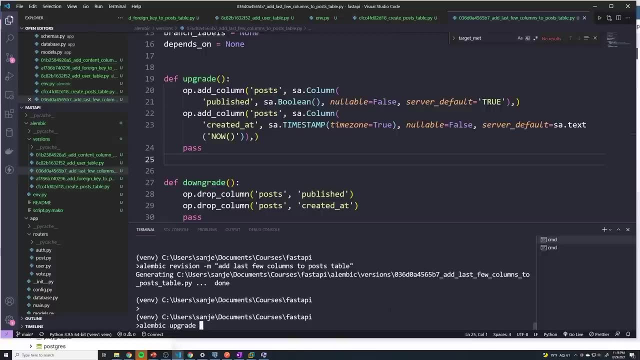 code And let's create a column and we'll just go. instead of doing head, we can just do plus one, just to show you guys how it's going to do the same thing in this case, And so it looks like it ran that And. 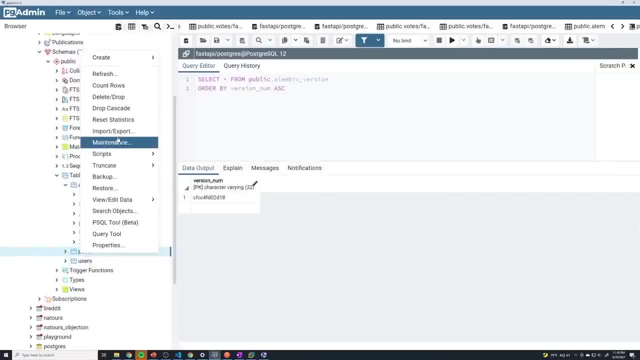 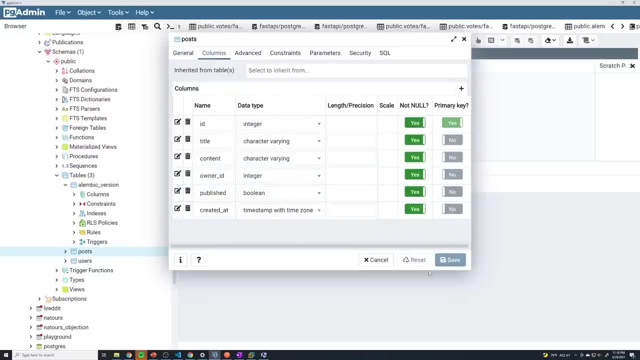 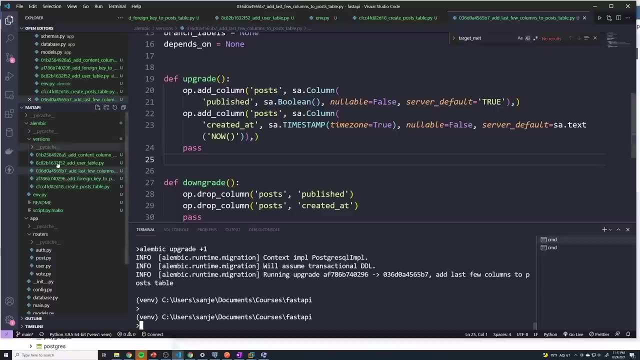 if we go back to Postgres, refresh this and then go to properties, we should see we've now got our published and our created at columns All right. And once again let's say that maybe we want to roll back right, Maybe we want to roll back all the way to back when 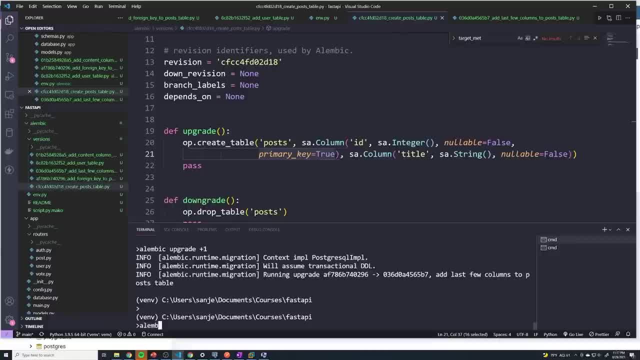 we just created the post table. You know we can once again do Alembic downgrade and just provide the revision number of the specific revision you want to go to. So we can go down to add user table, we can go down to create post table. we can go down to any section. 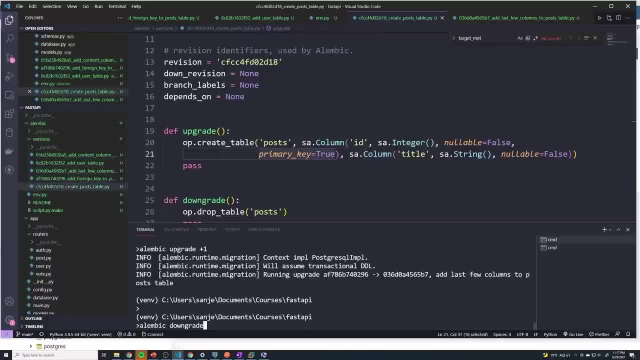 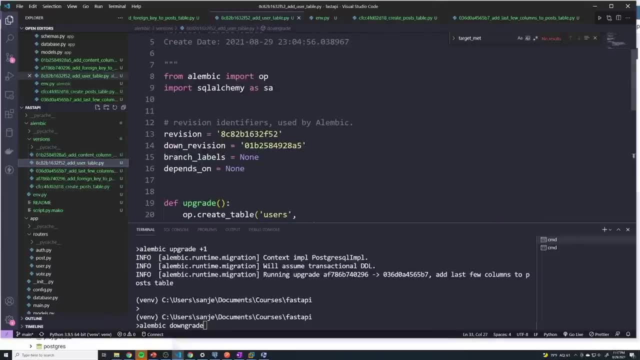 we want And it's really up to you. And so let's say: this time let's just go all the way down to, let's go down to add user table. So whatever revision this is, We can do that, All right. And so it deleted a whole bunch of stuff. It looks like it deleted. 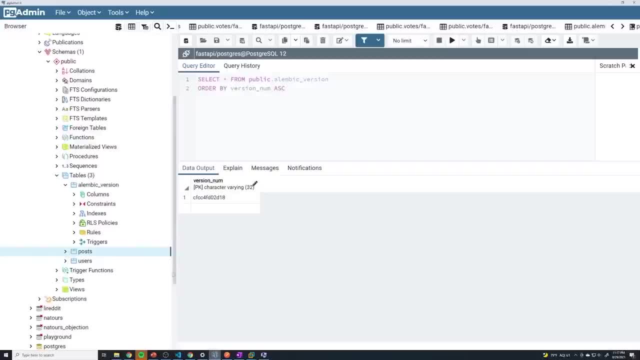 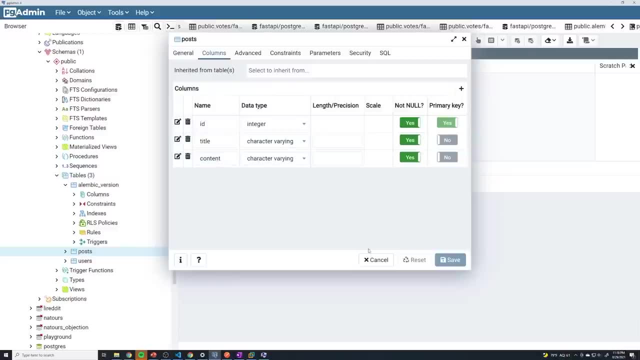 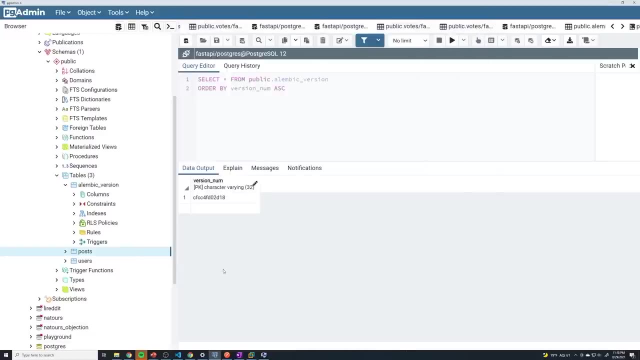 the last few columns that we just added, as well as the foreign key constraint, And so now if we refresh these tables, you can see that posts it doesn't have the extra columns we added And the constraints- foreign key- no longer exist. But fortunately we can upgrade. 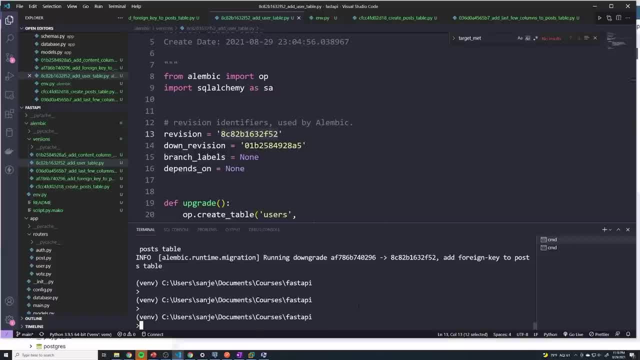 to a newer version, To one of the more recent versions. so I can do Alembic upgrade plus one. So if I do this it's going to go up one newer revision. So right now we're at the add user table And 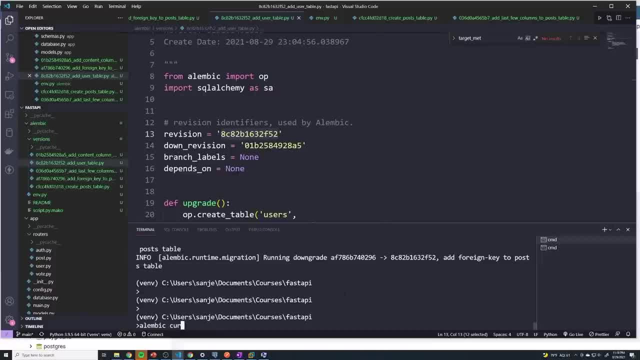 if you forget wherever you are, you can just do Alembic current, Right. so we're on 32F52.. And so if I do an upgrade right, we're going to go up to. I think we're going to go to. 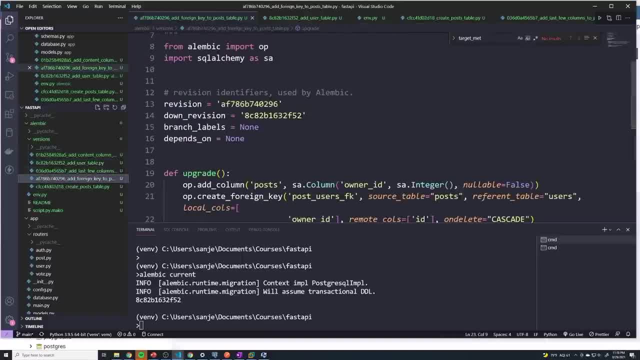 296.. I think it's this one, Because you can see that in this one, this revision is 296.. But the previous revision is 252, which is the one we're currently on. So I can do Alembic upgrade plus one, All right, And so now we've added the foreign key, If I do Alembic current. 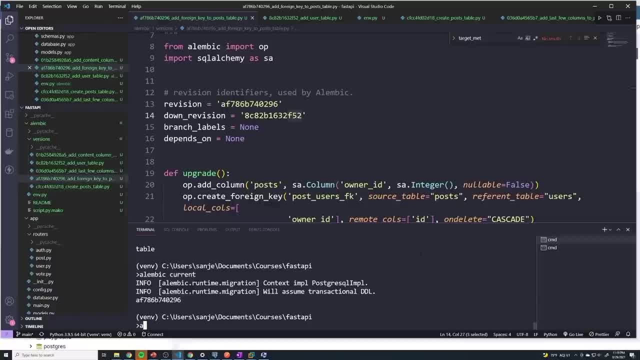 we can see that we're on 296.. And then if I just do Alembic upgrade, Alembic heads, it's going to show us, whichever one's, the latest one, which is 5B7.. So we can just go upgrade. 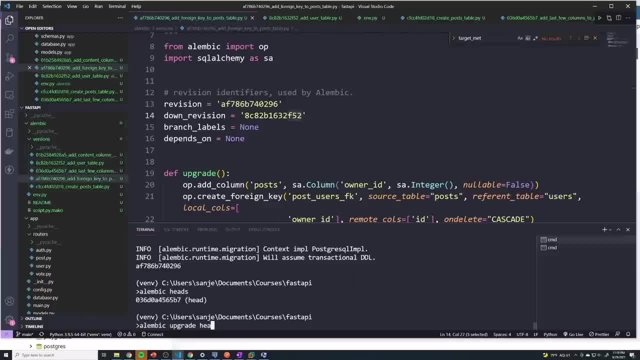 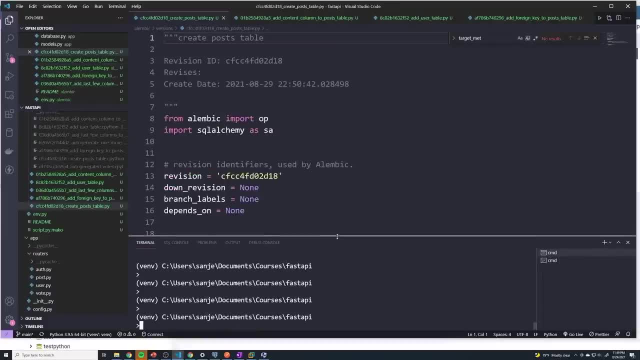 directly to that By doing head. The last thing that we have to do now is generate the votes table, but I'm not going to manually create it myself this time. Instead, I'm going to make use of the auto generate feature. So this is what I was talking about earlier. 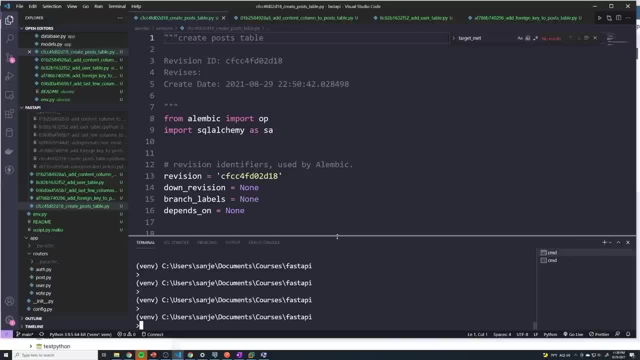 how we can use Alembic to be intelligent. We don't want to be intelligent enough to figure out what exactly is missing from our Postgres database and figure out what needs to be created. And the way it actually does that is: it takes a look at all at all of our models, So it's going to import all of our. 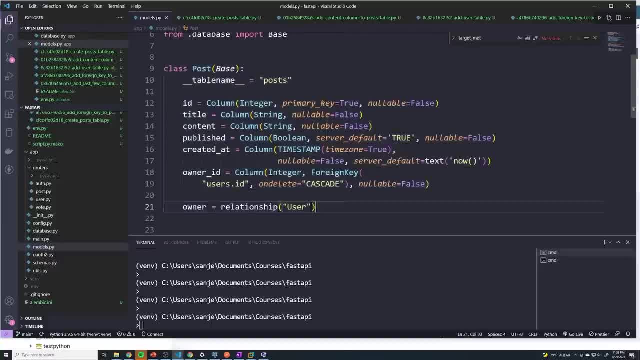 sequel alchemy models And, based off of the columns that we have set here, it's going to figure out what our Postgres database is is supposed to look like, And, regardless of what the our database is in its current state, we don't need to actually delete everything. 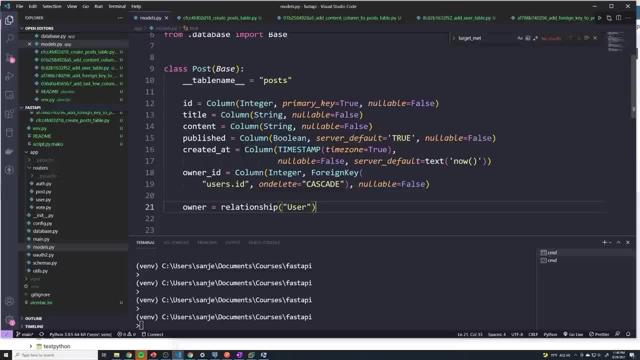 and build it from scratch. Instead, Alembic is going to be intelligent enough to figure out what columns are missing, what tables are missing, what extra columns do we currently have that we may need to remove, and it's going to figure out what's different between. 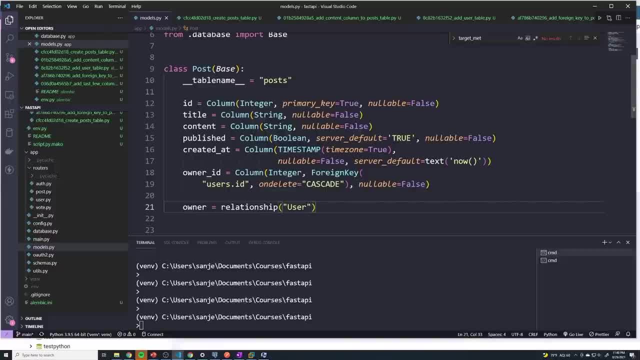 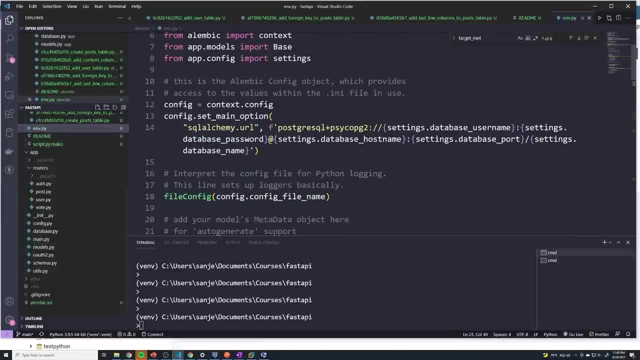 sequel alchemy models and our Postgres database and it's going to make the necessary changes for us. And so the way to do that, and first of all, I guess just to kind of reiterate the reason we can do that, is because we imported the models and then we passed it into this. 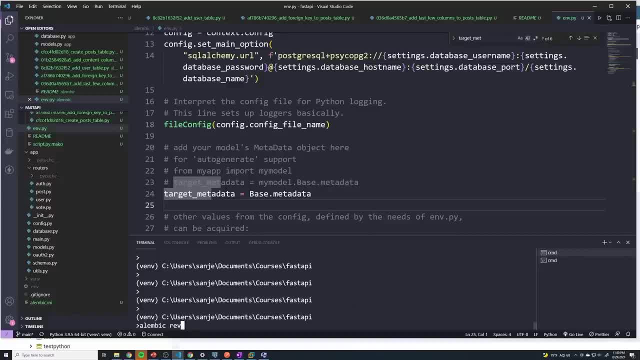 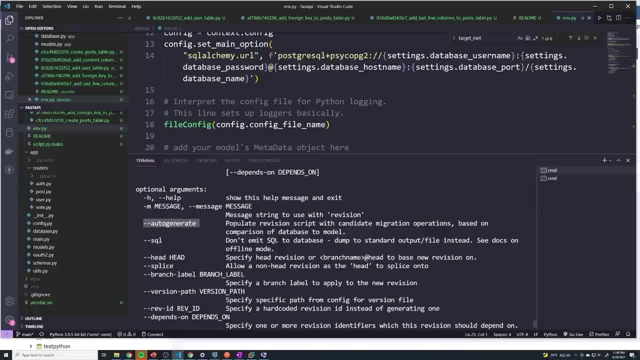 target metadata. So let's run Alembic And we'll do revision. But if we do dash dash help, you'll see that we're going to use one of the flags that we have never used before, which is the dash dash auto generate. So we'll do dash dash auto generate And then we will. 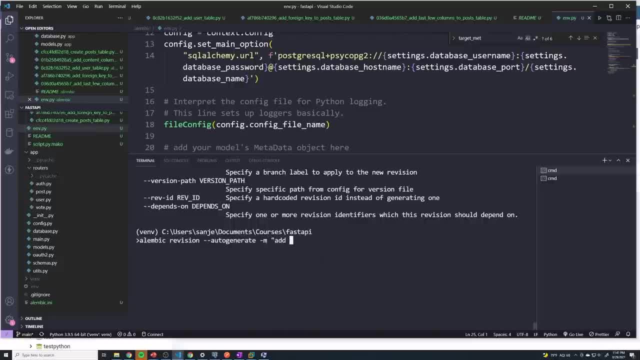 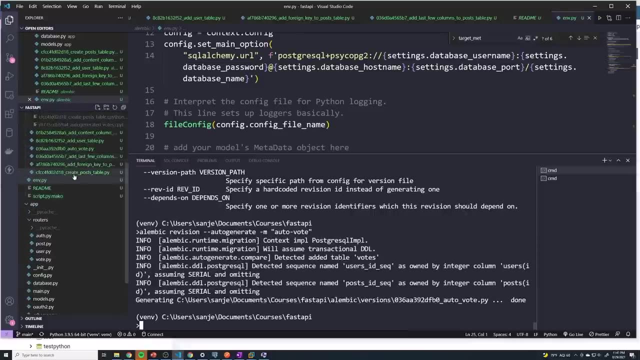 send a message once again. we'll say: add votes about auto vote, maybe because it's auto generated And I know it's going to add the votes table because that should be the only difference that we have. So we'll run that. 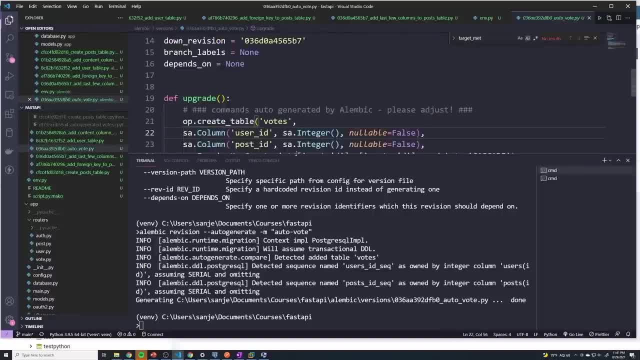 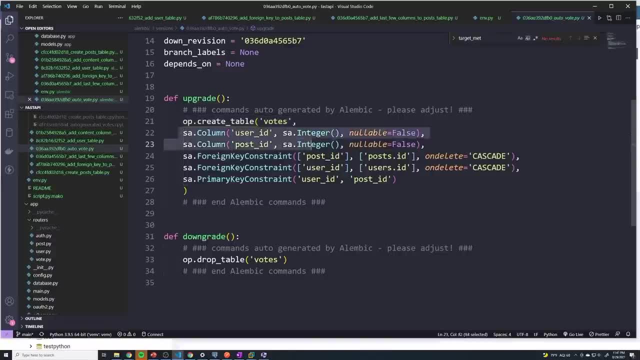 And so, if I go to auto vote, let's take a look at the changes it's going to make And so you can see here the changes where it looks like it's going to create the votes table. like I predicted. it's creating the two columns and then it's going to add the 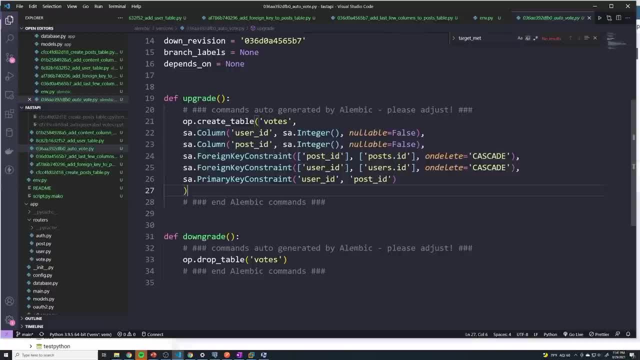 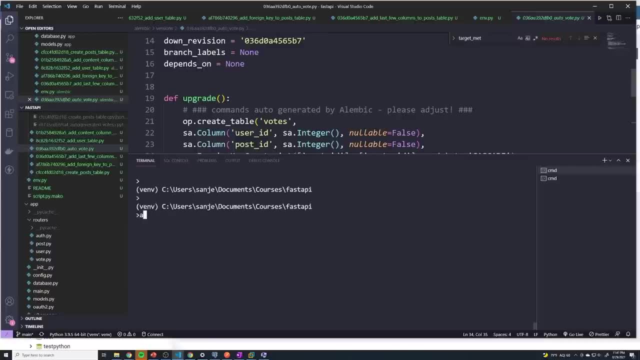 primary key constraint, as well as the two foreign keys as well, And it's going to even add in all of the on delete properties and things like that. Alright, and so all we got to do now is do an Alembic upgrade head. And now, if I run, 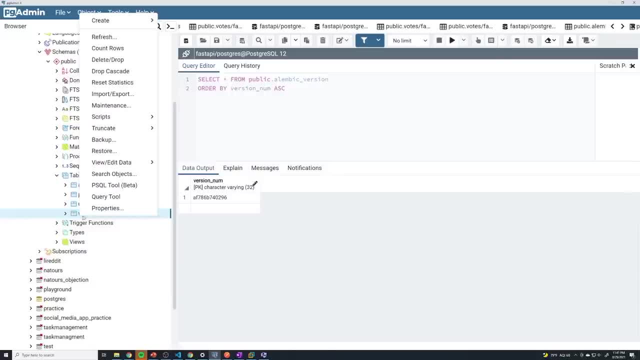 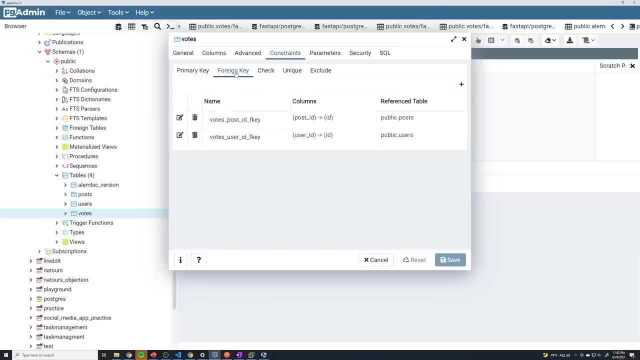 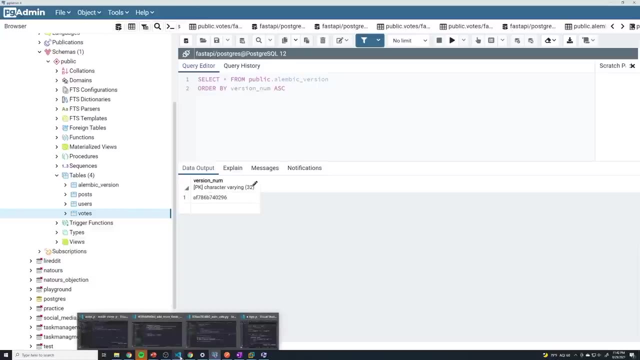 refresh this and go to votes and properties. right, we should have the two columns and then our constraints and foreign keys look pretty good. Everything looks set, And so that's how easy it was. So, no matter what state your databases at any point in time, 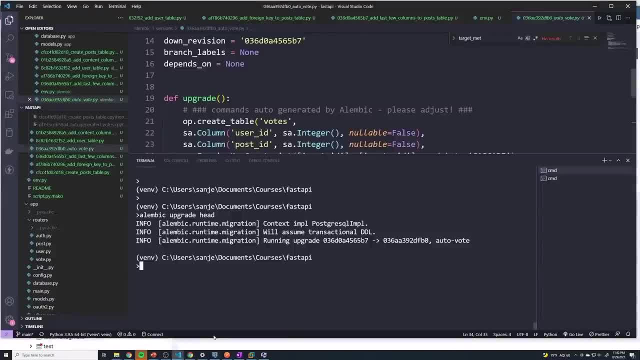 you can, all you can always do the auto generate functionality to get it back to a state that your code expects it to be. And the best part about this is moving forward. let's say, I want to go back to my models and I want to change something, So I've got. 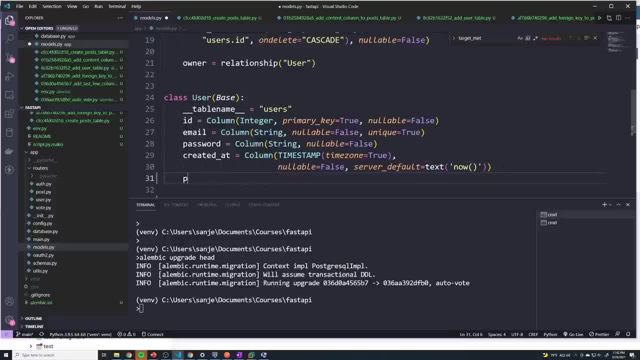 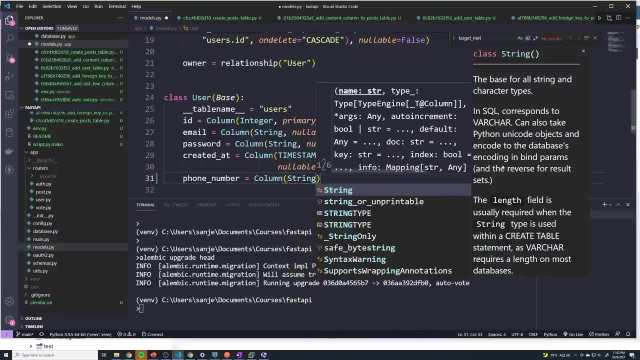 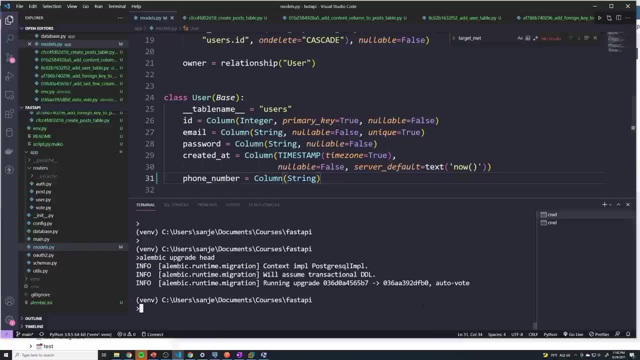 my user model. this time I'm going to add that phone number column And this is going to be string. Alright, so any changes we make, even on a table that already exists, what we can do now is I can do a revision, auto generate. 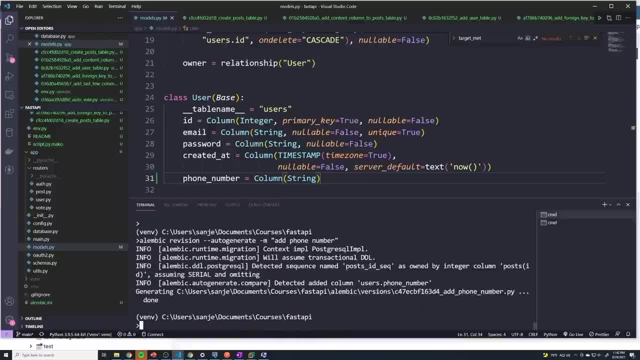 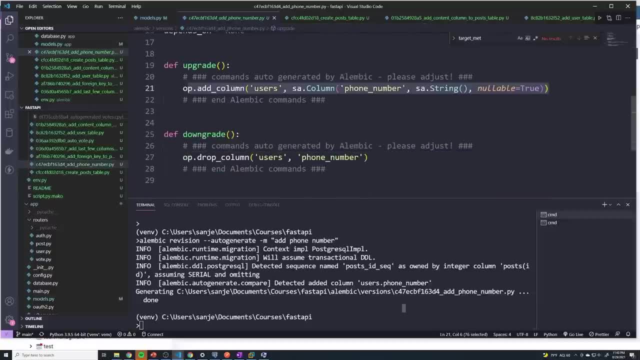 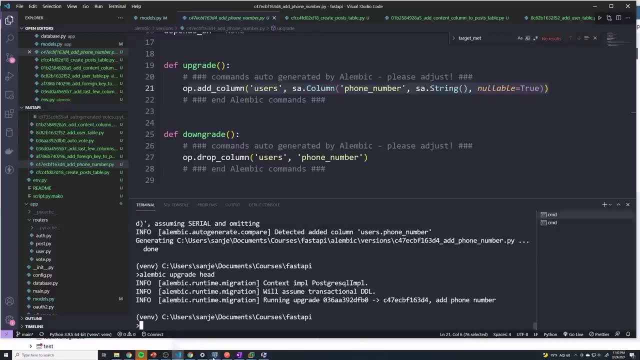 Here. I can just call it: add phone number. All right, and then if we go take a look at that, we can see that, hey look, we added our phone number column, And so the only thing else we have to do is do an Alembic upgrade head And it's going to push out those changes. So let's 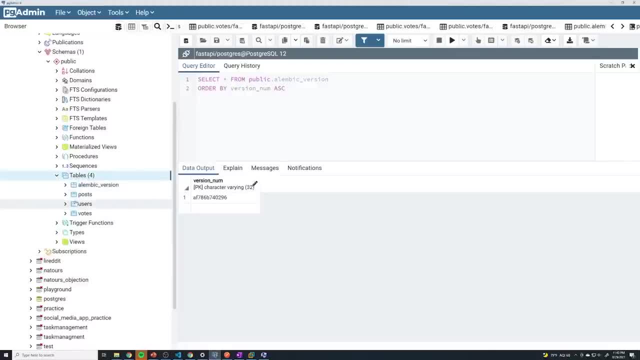 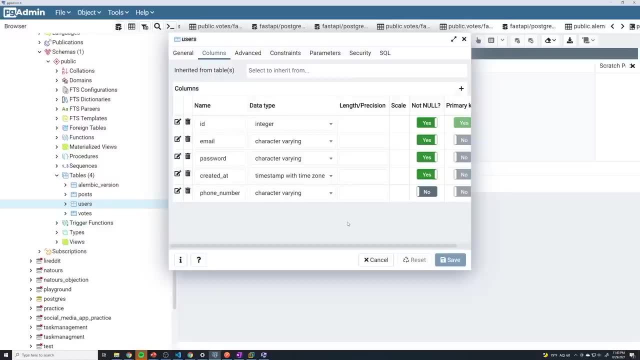 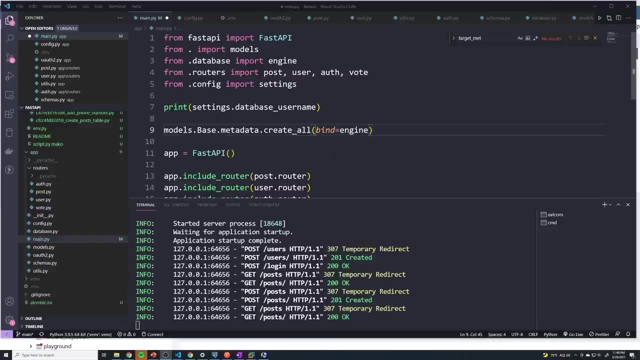 refresh this And let's just double check. We go to users now properties. we can see phone number column is now set And I think that's pretty much going to wrap up at the top, And then we can go back to what we had in the beginning And we can go back to our 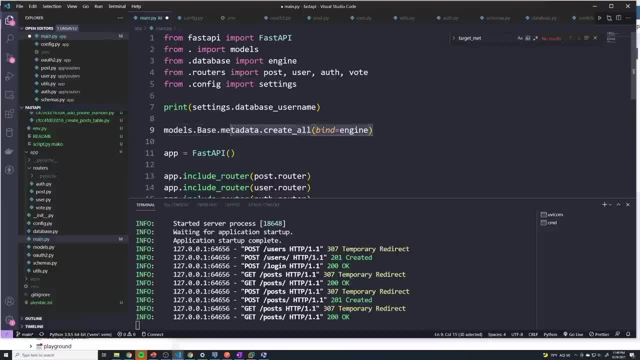 old page And this is going to take us back to the old page. So let's go ahead and go back to the old page And let's just check that out. Alembic migration isn't going to have to do anything because everything is already there. 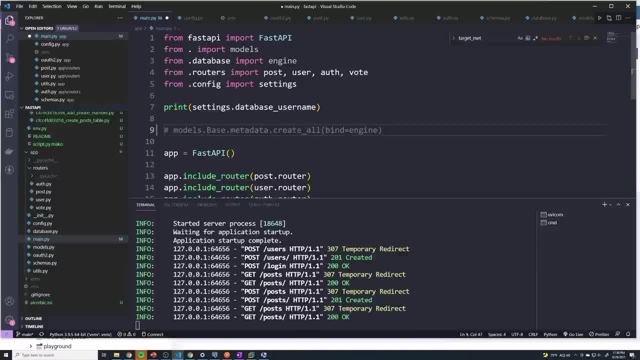 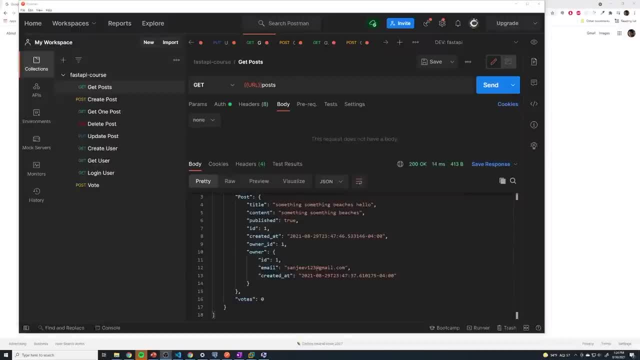 But I'm going to leave this commented out moving forward, because I don't really need it And it's really up to you guys for what you guys want to do. For the most part, throughout this course, we've been testing our API by sending a request from postman, And postman is a great 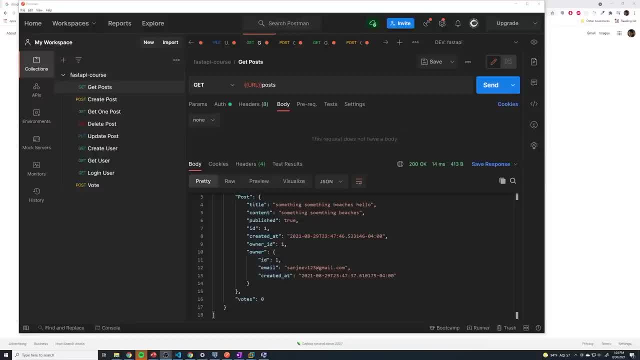 tool. But there's one thing to note, And that is that when you send a request from postman, you're actually sending a request from your own computer, And it's important to understand this, because your API can get requests from different types of devices. you can get a request from a. 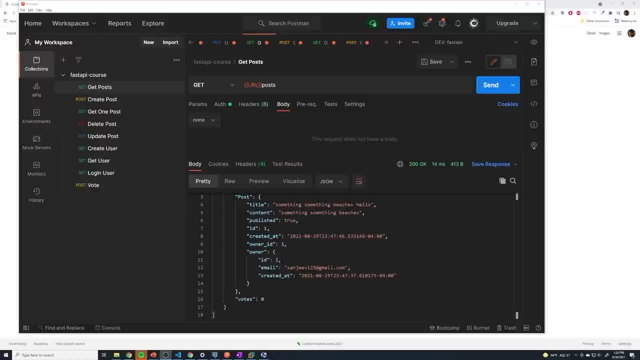 computer or a server, whether that through postman or even through curl- If you've ever used curl, it's essentially doing the same thing that postman is doing. it just doesn't have a nice little guy- can also get requests from mobile devices. But, more importantly, you can get requests. 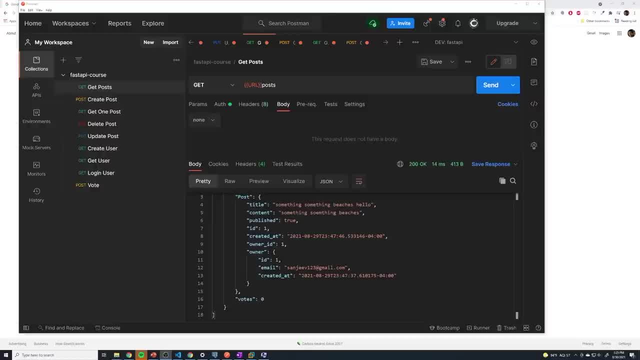 from a web browser. So when a web browser sends a request, you know, using JavaScript fetch API, there's going to be a slightly different behavior that we have to account for, which we can't take into consideration when sending requests with postman, because 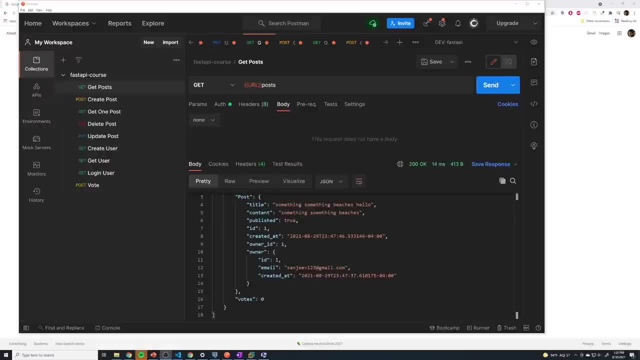 postman is going to use JavaScript to allow what you know in JavaScript as a request to get a is request from a web browser. So when a web browser sends a request, you know, using Javascript fetch API, Postman isn't a web browser. So what I'm going to do is I'm going to show you exactly what happens. 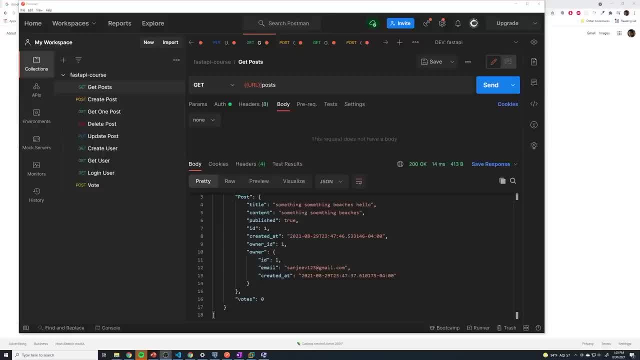 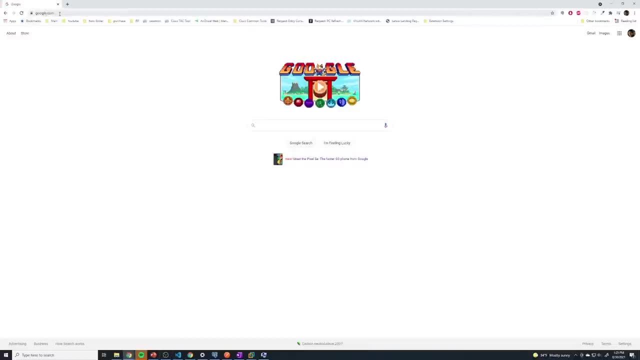 when we send a request from a web browser instead of our own computer, using Postman. So what I want you guys to do is open up your web browser and specifically go to googlecom. It's important that you go to googlecom, or technically, this is going to work on any website. 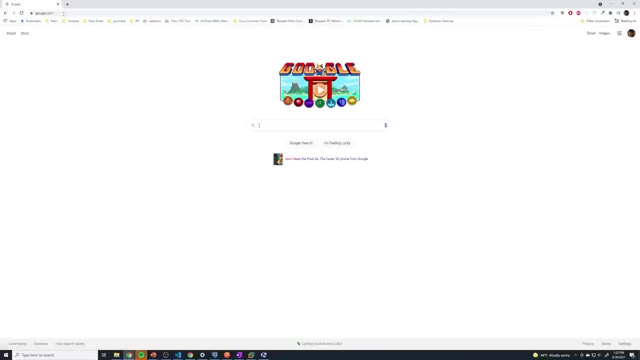 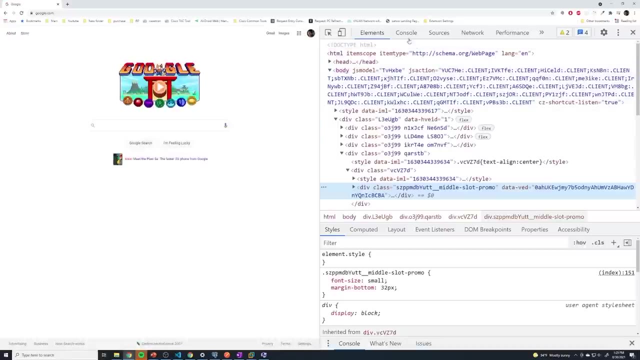 but I need you to actually go to a specific website like googlecom, And then I want you to right click on the web browser and just hit inspect. So this is going to open up the Chrome developer tools, And if you aren't too familiar with it, don't worry, It's just a. it's a built 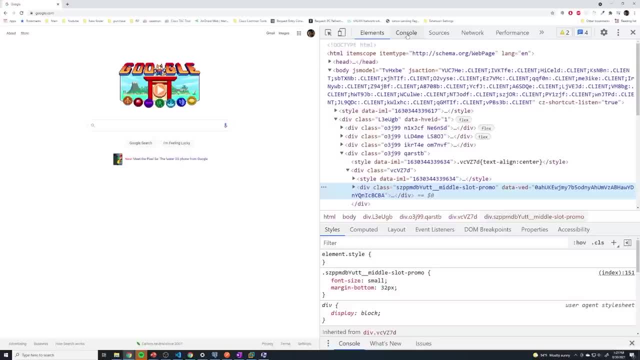 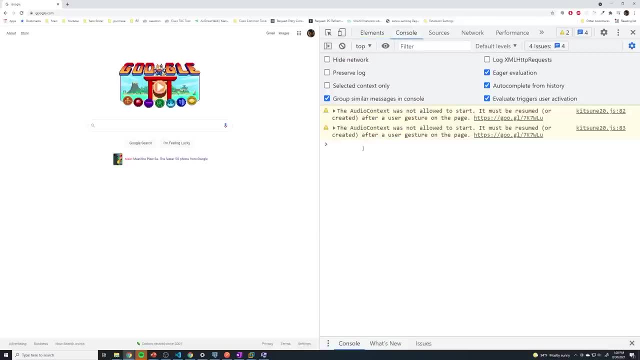 in tool to that we have in Chrome or any web browser that allows you to make. it makes it easier as a web developer to kind of troubleshoot things. But what we can do is if you go to console, we can actually send an API request to our API from googlecom or from our web browser. 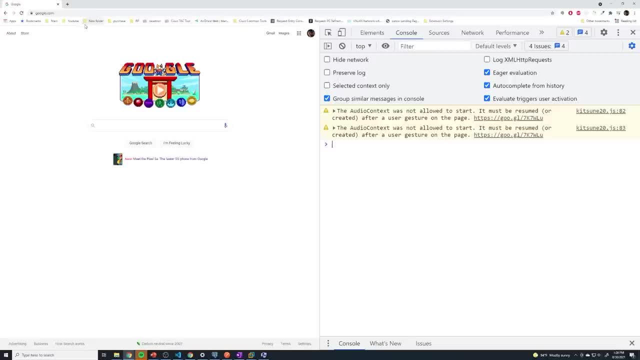 which is on the googlecom domain at the moment, And so I want you to just type this in: we're going to say fetch, So this is how you perform an API request from the web browser level, And we're going to send a request to our fast API. 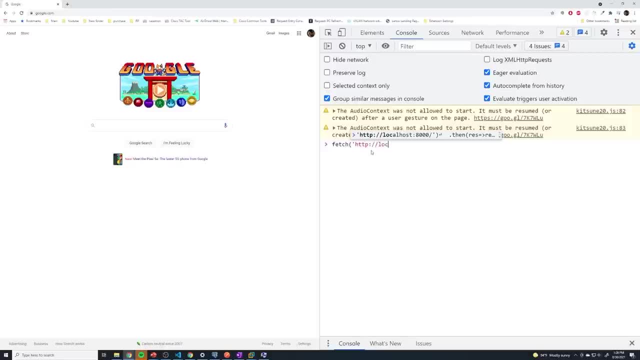 So that's going to be hosted on HTTP colon slash slash, localhost, colon 8000.. And then just type in then. So don't worry too much about this. but it technically returns a promise, So we have to resolve the promise. we just say res resjson. 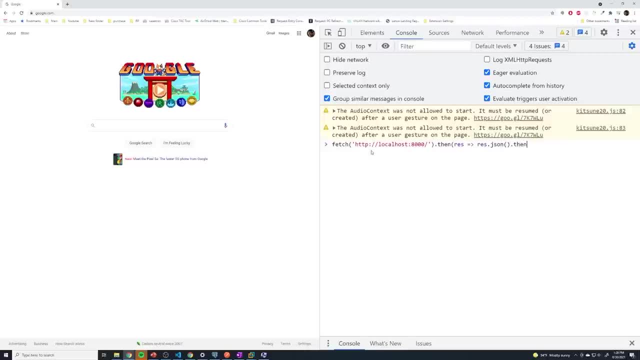 And then do another then and just say console, dot, log. And I forgot one bracket right here, And so all this is doing is it's sending a request to the root URL of our API And then it's going to print out the contents of whatever we get back from the server. So when I run this, I want you. 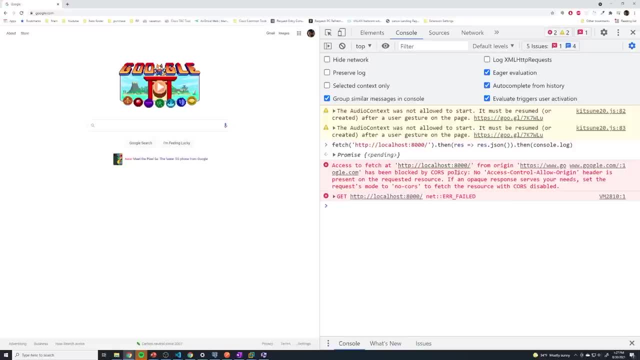 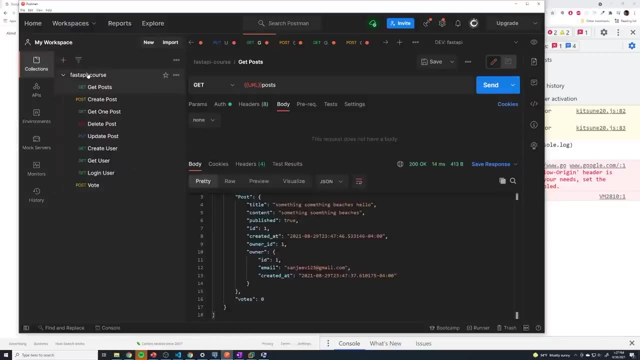 to notice something. we get an error. It says access to fetch localhost colon 8000 from origin and then it has: googlecom here has been blocked by cores. So what is happening here? Why is it that I can't send a request from the web browser, But if I go to postman and I just create a quick new request? 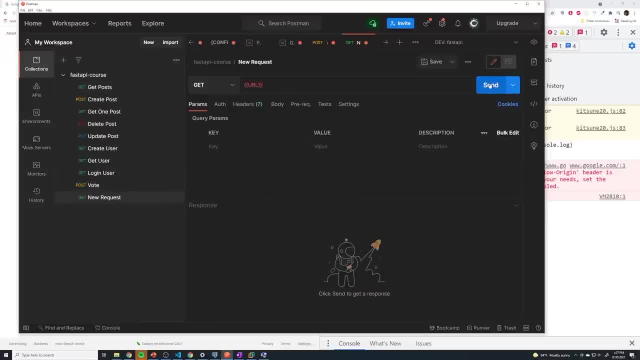 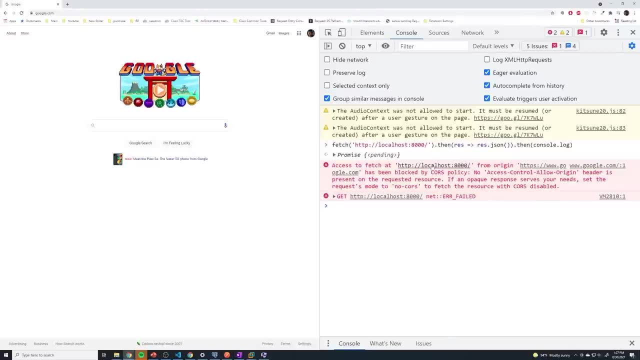 And we can just go straight to URL. It resolves just fine. Well, it has to do with this course policy. So in this lesson we're going to take a look at what exactly this course policy is and what we can do to. 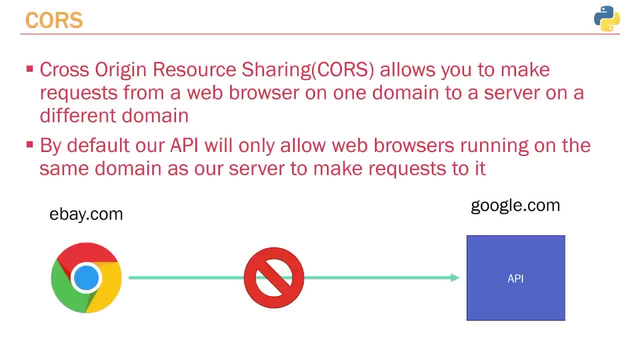 ultimately resolve this issue. So what exactly is course policy? So course is short for cross origin resource sharing, And so course allows you to make requests from a web browser on one domain to a server on a different domain, And by default, you know, when you configure an API, whether it's in fast API or any other framework or language. 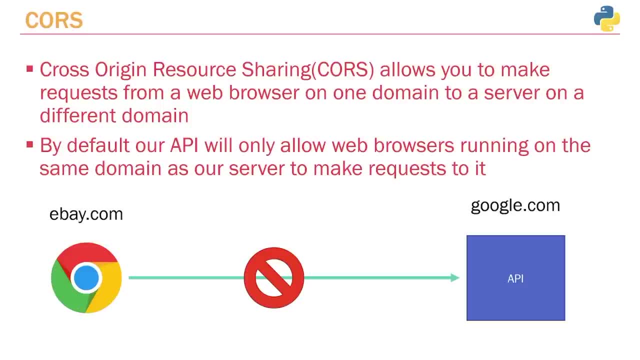 you will only be allowed to send requests from a web browser running on the same exact domain as your server. And so what exactly do I mean by that? Well, if our API is hosted on googlecom and our and our website is hosted on ebaycom, ebaycom, by default, cannot send a request to an API running on a. 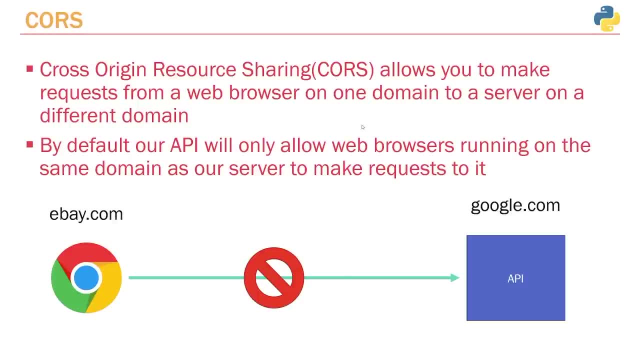 different domain like googlecom, it's going to get blocked by cores. However, if our web, if our website, was also running on googlecom and our API was also running on googlecom, then they'd be able to talk just fine by default. And just to prove that to you guys. 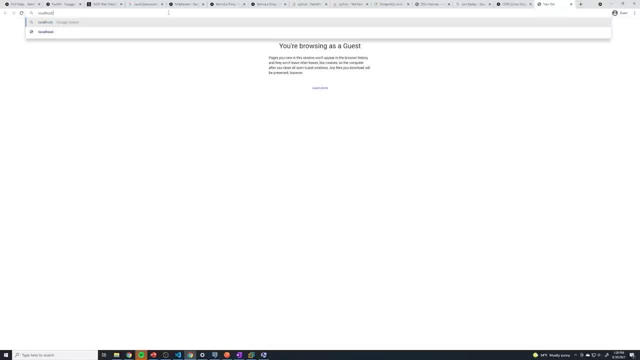 if we go to our web browser and go to localhost, colon 8000, you know which is the, the URL that our application is currently running on- you can see that I get a response back. So our web browser was able to make- and, by the way, when I 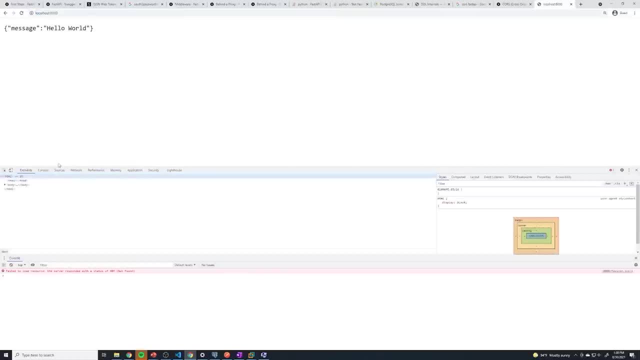 when I did this right. it did the same thing, as you know: going into Chrome developer tools and actually sending a request. And just in case you don't believe me, I'm just going to actually just show you guys, even on here. If I paste it, you can see that it was able to resolve and we 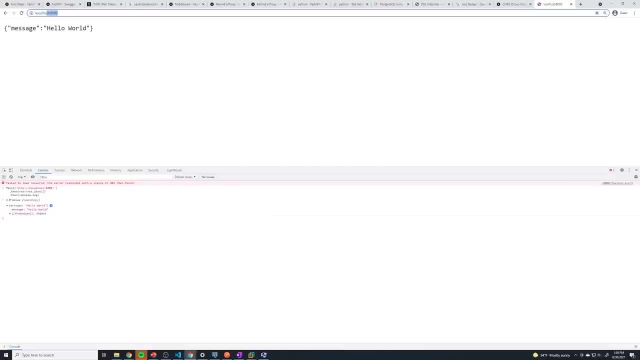 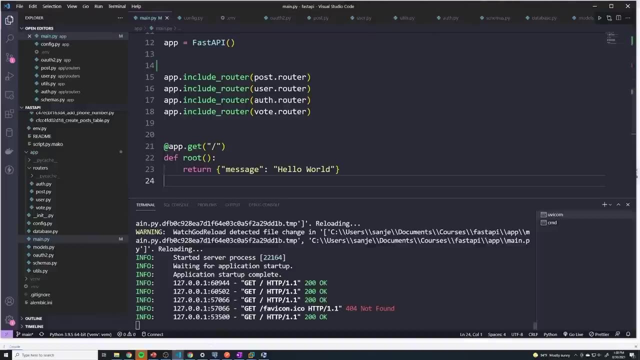 can see the hello world. So the reason why it works on this website is because this is the same exact URL or domain name that our API is running on right. our API is running on localhostcom, colon 8000.. So by default, they're able to talk to one another only when the web browser domain is. 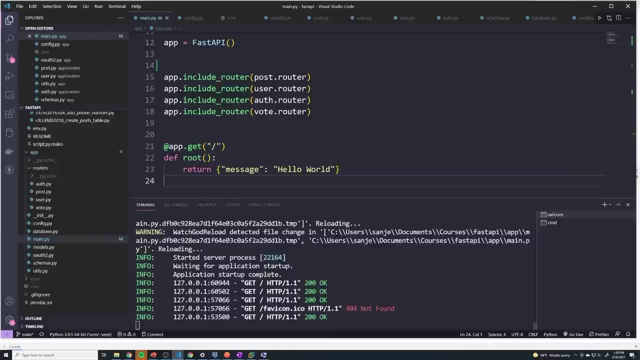 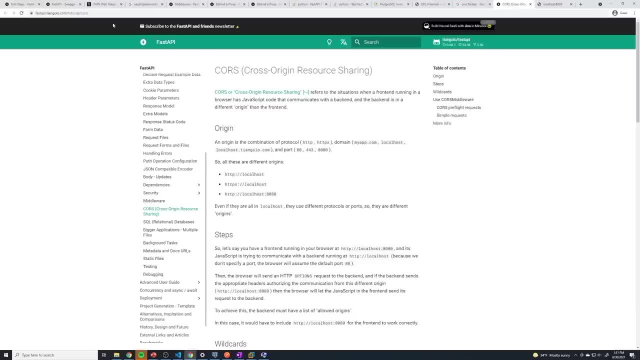 on the same exact domain as the API's domain. So to fix this, you know, if you did want to allow people from other domains to talk to your API out, what you can do is take a look at the fast API documentation and just search for cores, cross origin resource sharing And you'll see that. 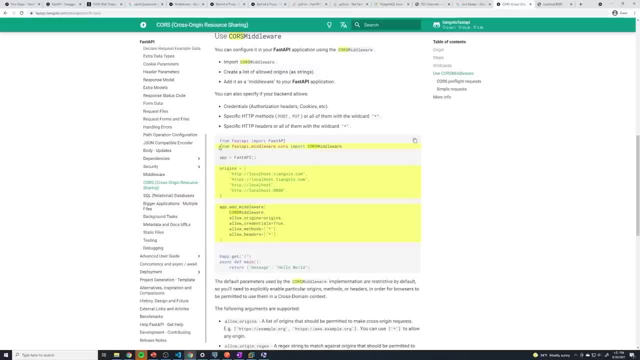 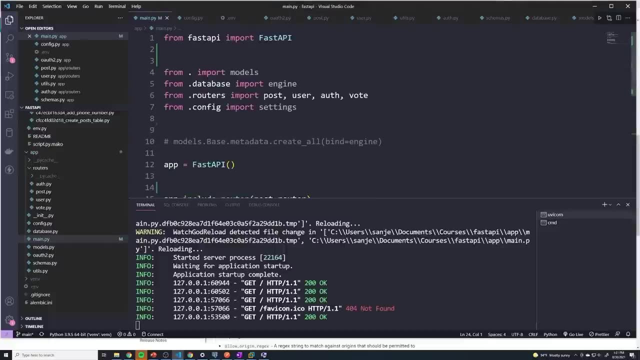 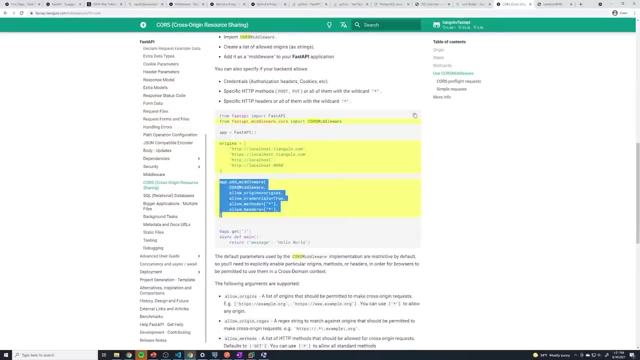 setting this up is really simple. So the first thing that we have to do is from fast API middleware cores. we're going to import cores middleware, All right, and then just copy this section right here And I'll explain line by line exactly what each one is doing. And so, under the app right here, 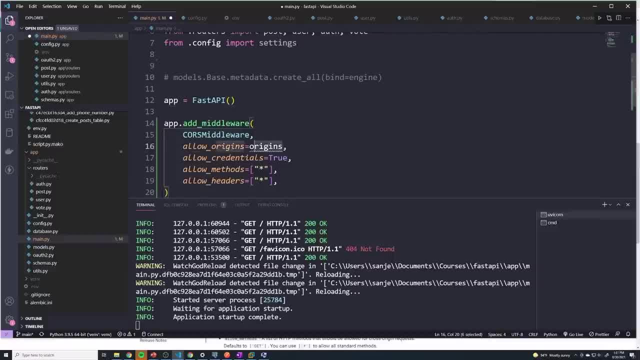 we'll just paste this in And it's gonna throw a little error here, but we'll come back. you can actually delete that and change that to a an array for now. But what we want to do is, first of all, we have to pass in the 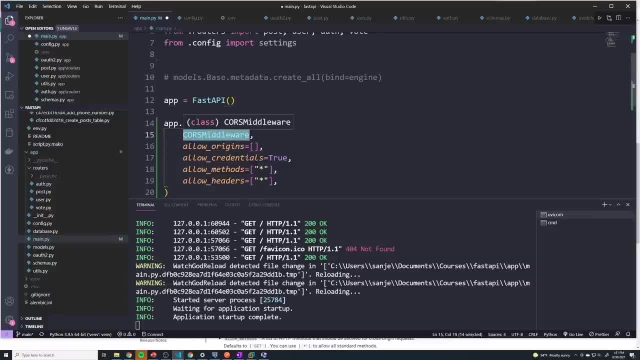 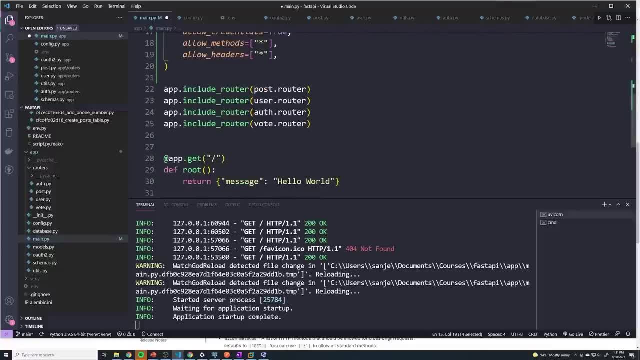 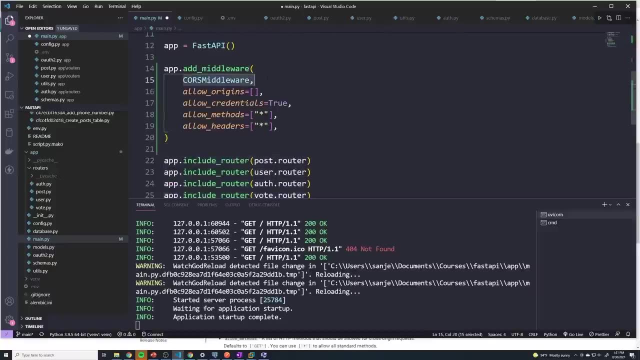 middleware, And middleware is a term that's used in most web frameworks because it's basically a function that runs before every request. So if someone sends a request to our app and before it actually goes through all of these routers, it'll actually go through the middleware And then our middleware can perform some sort of operation. 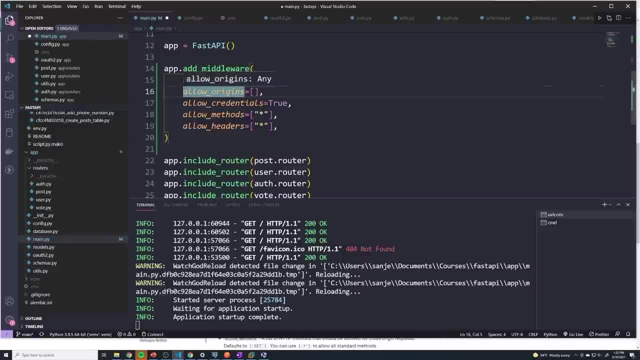 But what we want to do is, first of all, we have to specify the origins that we want to allow. So what domains should be able to talk to our API? because right now it's only it's no domains- only if it's running on a. 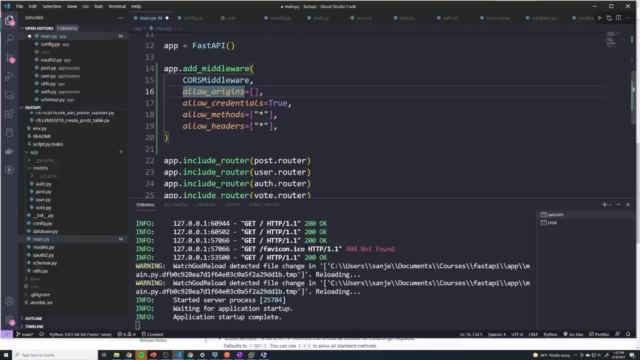 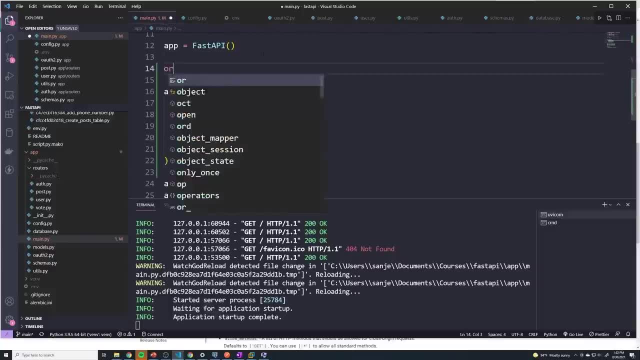 same exact domain, are you able to talk to our API? So the way we can do is we can put in: we'll create a list called our origins And I'll say origins equals, and it's just going to be a list. And here we're going to perform, provide a. 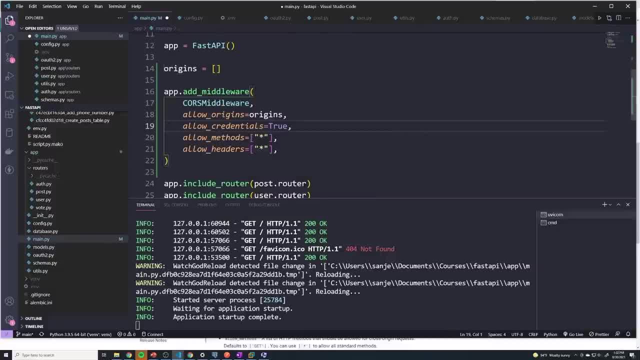 list of all of the domains that can talk to our API, And before we fill that in, I just want to quickly talk about the other three as well. So our cores policy can be pretty granular. So not only can we allow specific domains, 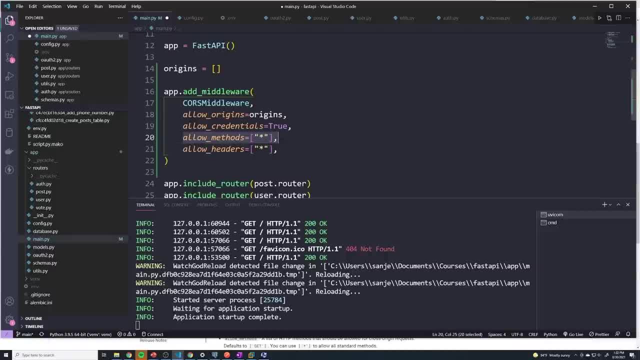 we can also allow only specific HTTP methods. So if we were building like a public API where people can just retrieve data, we may not want them to allow, we may not want to allow them to send, post requests and put requests and delete requests. So we could potentially just allow get requests And then we can even allow specific headers as. 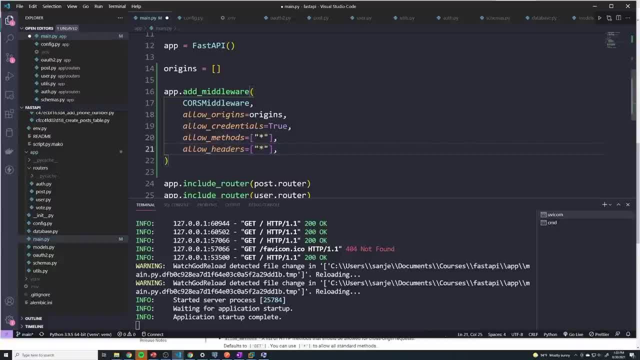 well, But for now we're just going to allow all headers and all methods And we're going to just kind of drill down based off of what origins can talk to us, And so you know if we want Google to be able to talk to us. 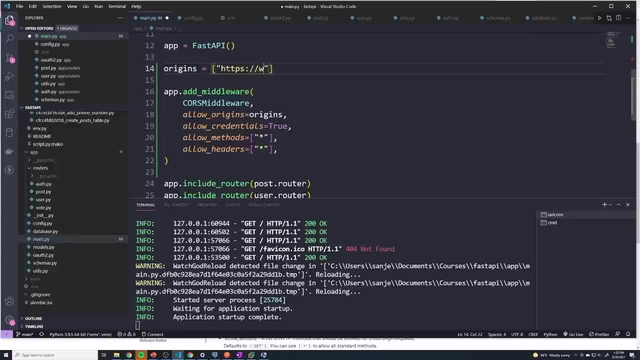 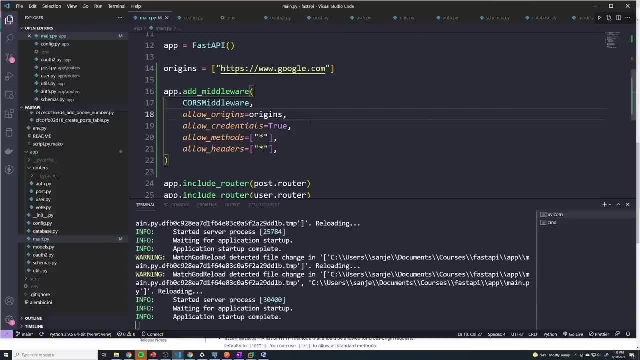 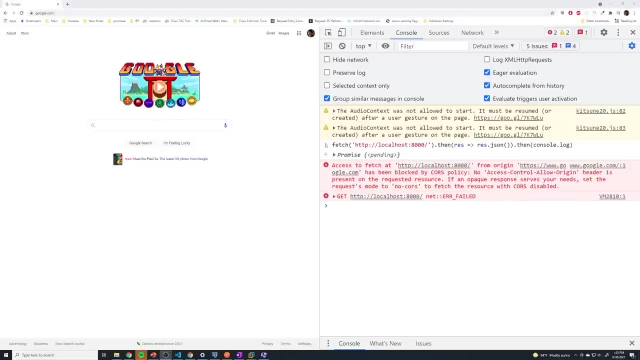 I can just say: HTTPS, colon, slash, slash, wwwgooglecom, And so now this course policy is set to allow people from googlecom to talk to us, And so if I go back to googlecom, I just hit the up arrow so I can run this command again. you'll see that I do. 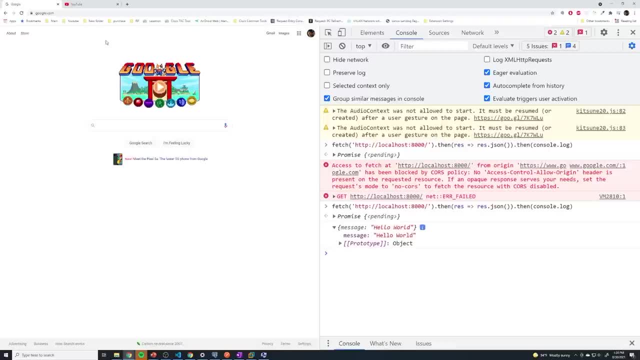 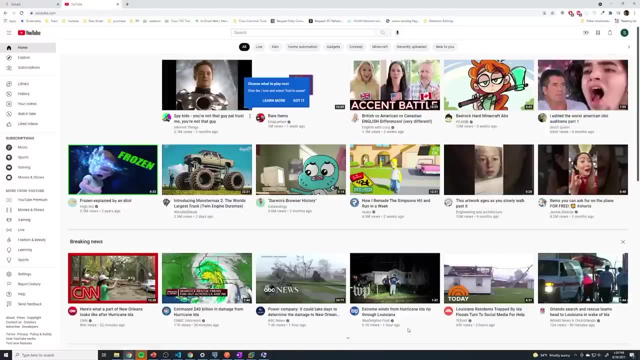 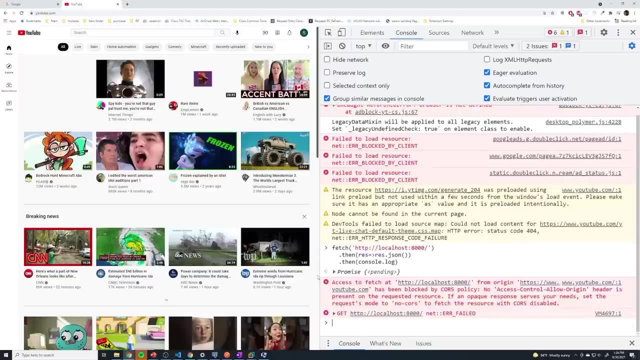 successfully get a response back and there's no core there. However, if I go to a different website- so you know some website on a YouTubecom And then we go and then we send the same exact request from the console- We once again get the course error And 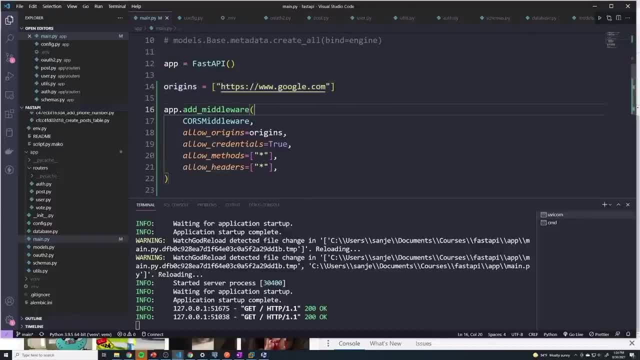 that's because in our, in our list of origins, we're not providing wwwcomyoutubecom. So if you wanted to also allow youtubecom, then we'd have to do HTTPS colon slash. slash- wwwyoutubecom. For now, I hit the up arrow. 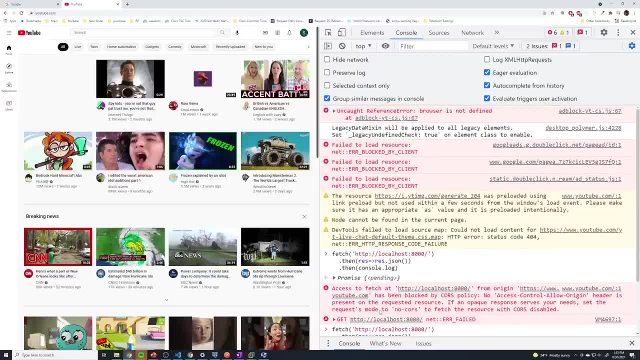 And then we hit the up arrow And here we go. We can see that it properly resolve. So you just have to provide the list of URLs that can talk to your API, And if you want to set up a public API so that everyone can access it, then your origins would just be a wildcard. So this: 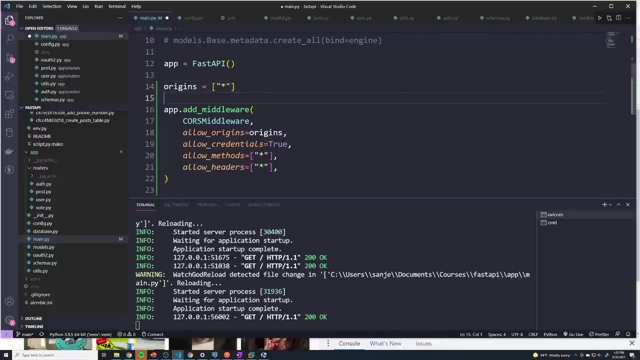 means every single domain or every single origin, But if your API is being configured for a specific web app, then you definitely want to make sure that you provide a strict list of origins. So just one of those: whatever domain your, your web app is running on, so that no one else can you know accidentally. 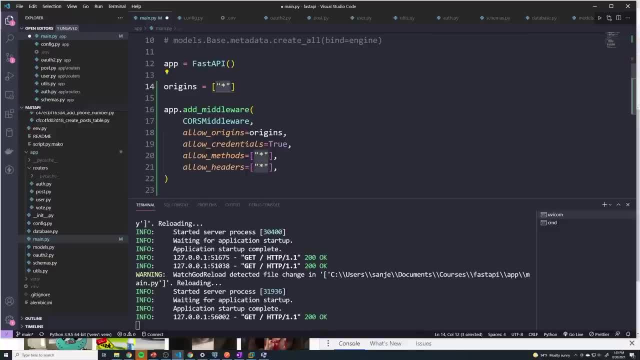 reach our application for some reason or another. It's just security best practices to really narrow down the scope of the origins that can actually access your API. For now, I'm just going to leave this as a set to everyone so that you know when we actually go to deploy this. 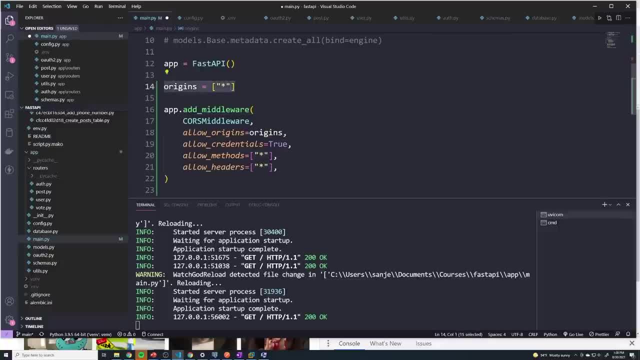 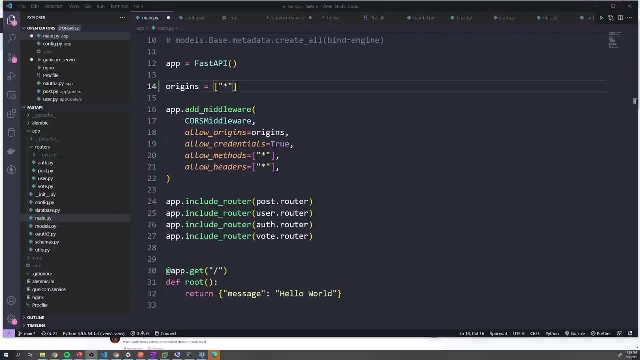 it'll be a little bit easier from a testing purpose, But feel free to update this accordingly. In this lesson, we're going to focus on setting up Git for our projects so that we can start tracking our changes, as well as set up a remote repository to store all of our code. 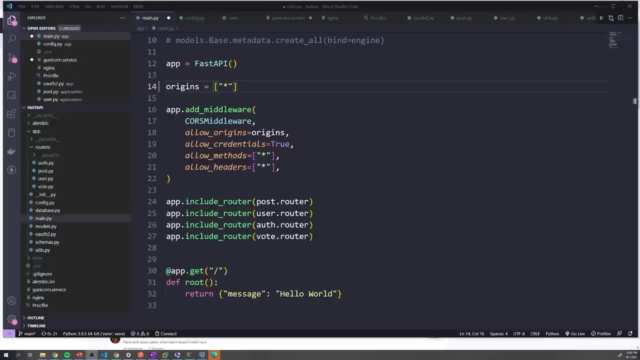 This is going to make the whole deployment process a whole lot easier. But before we set up Git, there's a couple of things that we need to do, Because when you check your files into Git, by default it's going to check in all of your files And there's going to be some files that 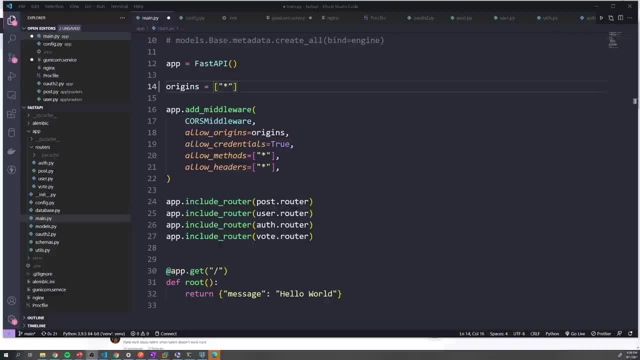 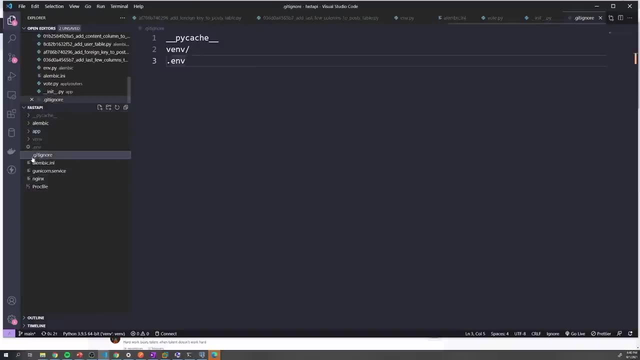 you don't want to be uploaded to a remote repository or even into your Git in general, And so we have to create a file called a git ignore file. And so if you go to the main root, root folder of your project, I want you to create a file called dot git ignore, And it's important that you put 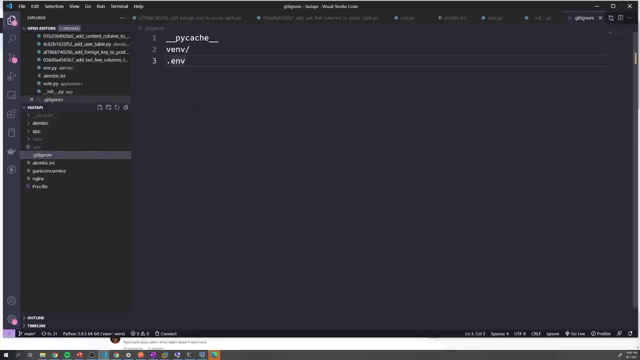 the dot in front of it. So it's dot, git ignore, And so this file is going to tell Git what are all of the files and folders we don't want uploaded to Git, And so some of the common things that you would not want to be tracked within Git is going to be your dot env file, So this is going to be. 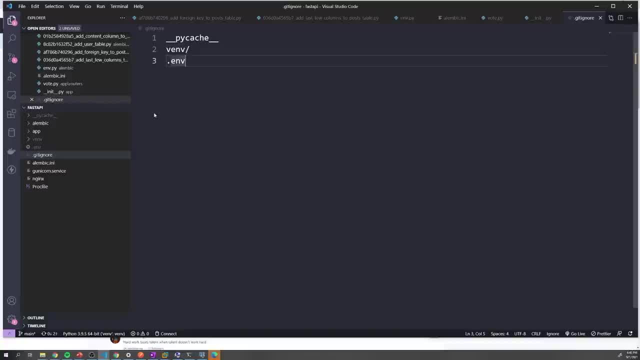 all of your environment variables. Obviously, you don't want to check those in, or then you know, if this is part of a public repository, then anyone can see those. But also on top of that, you'll see all of these random. 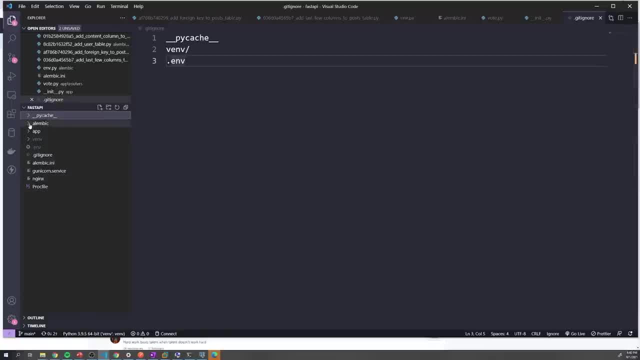 pi cache these underscore, underscore, pi cache folders. So I'll go ahead and add that in there as well, because we don't actually need to check that into Git. And then, finally, we have our folder which contains our virtual environment. We don't want to check that in as well, just because 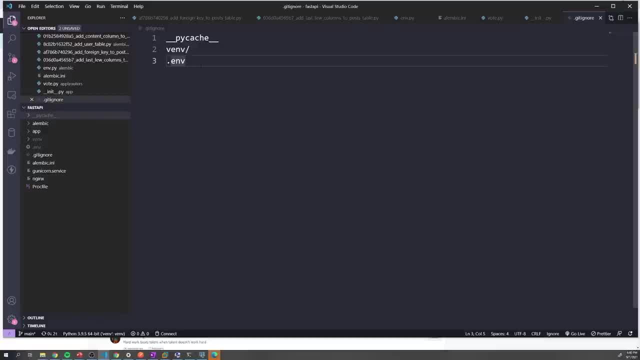 we have no idea if someone else who wants to clone our repository is going to be using a virtual environment And if the end. if they are, then we're going to have to check that in as well. So let's go ahead and click on that. So we're going to click on that and we'll see that. that's. 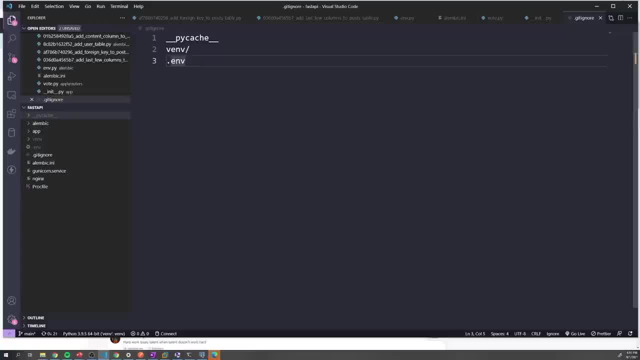 going to be our folder, And then we're going to have to load it from our drive, So we'll be able to see all of that here. And then we have our virtual environment, And if we want to actually to actually upload a folder to our virtual environment, it just wouldn't make sense. And on 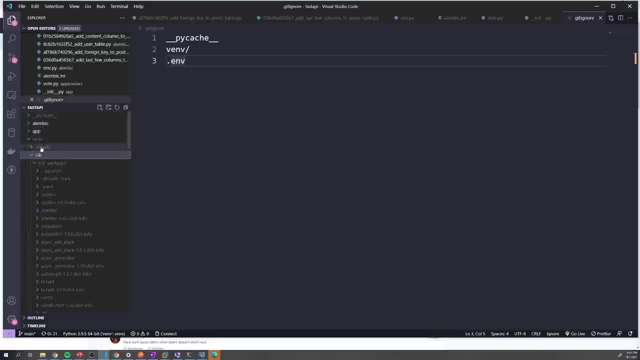 top of that, our virtual environment contains all of the third party libraries that we've installed, So all of the different packages we installed through pip, including fast API itself, So all of the code of fast API, is within that virtual environment folder, And so there's no. 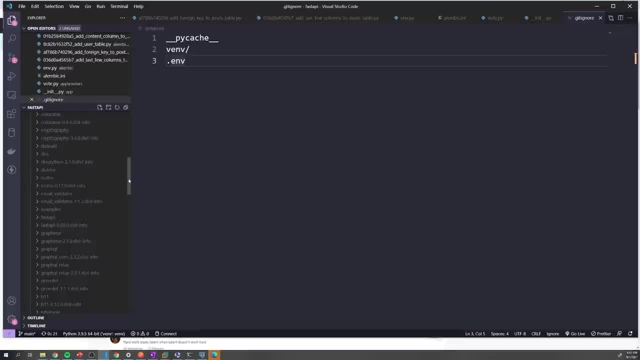 need to actually upload all of that, because that's a lot of a lot of files that actually take up a decent amount of space and it just wouldn't be efficient to actually upload those to Git. However, this does create one bit of an issue Because if we clone the repository at this point right, we have no idea what packages we need to install because our virtual environment didn't get uploaded with it. So we need a way for other users, other people on our team, to know what packages and dependencies we need our application, so that our application actually works. 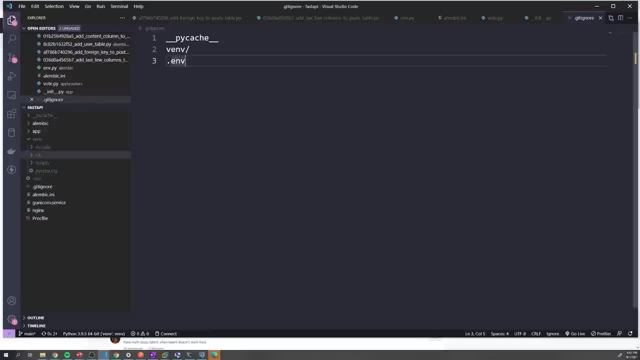 And so the way that we actually do this is well. first of all, before we even proceed, go ahead and copy this into your git ignore file, And make sure you have this before you do anything else, Because once certain files get checked in, it's very hard to get them removed. 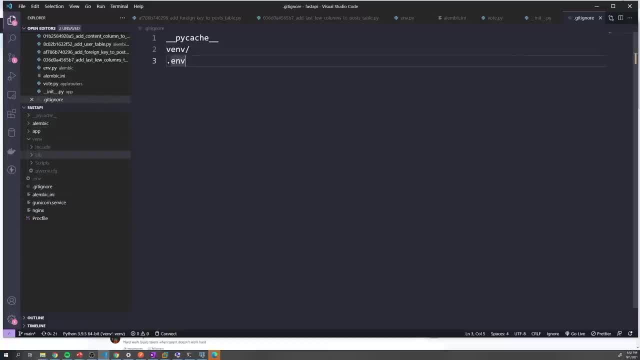 But after this, what we want to do is we want to create one more file and open up your terminal, And what we're going to do is type in pip freeze. So pip freeze is going to dump out all of the different packages and libraries that we have installed, as well as the specific version. 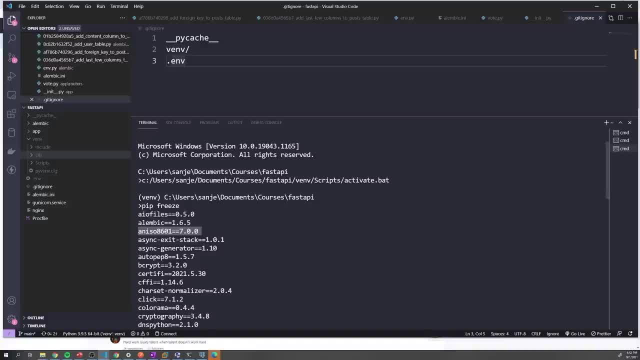 And so this is the information that we want to upload to git, so that, if anyone else clones our repository, they'll know the exact versions of every package they need to install. So what we're going to do is we're just going to take this output and we're going to pipe it to a file, And the file name is going to be called requirementstxt. 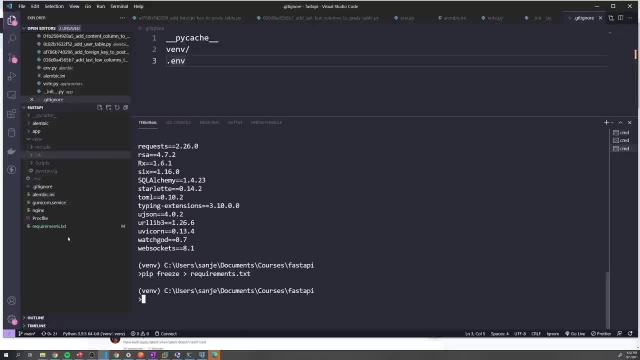 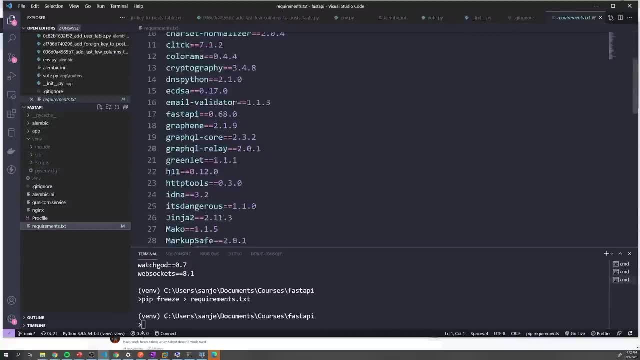 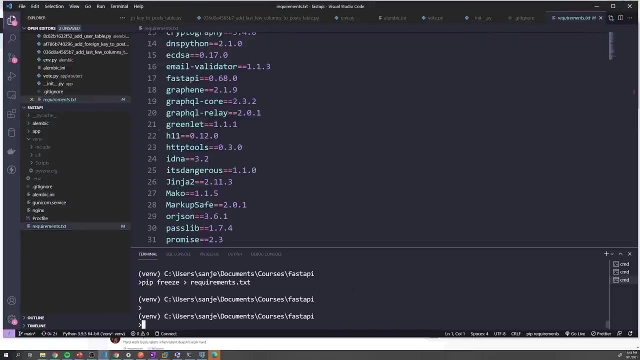 So this is standard convention With any Python application. you want to create a requirementstxt file that's going to contain the version of all of the different packages that you have installed, And so if we check this into git now, then anyone else can just take a look at a requirementstxt file and then actually install dependencies based off of what's in this file. And so for anyone else that clones our repository, all they have to do, instead of going one by one and installing these, they can just type in pip, install dash r requirementstxt, And that's going to install everything that's in this file. So this does simplify the process and it prevents us from having to upload all of those third party packages into git. 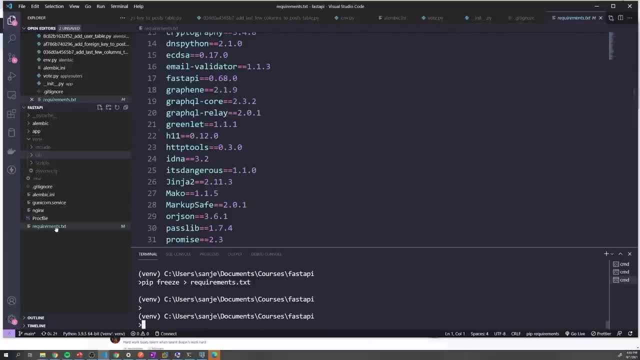 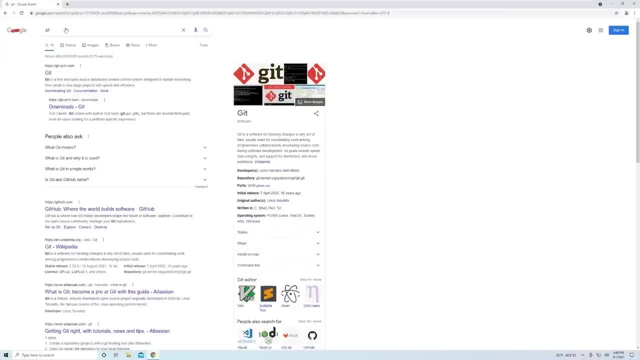 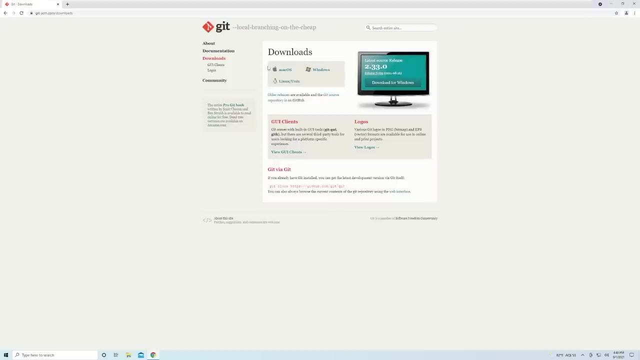 But we've got everything set up at this point. we've got the git ignore file and we've got the requirementstxt. So what we need to do now is actually set up and install git on our local machine. If you don't already have git installed, then in this lesson we're going to focus on getting installed on your local machine. So just search for git, And then you can either go to the main page or you can go straight to the downloads page. So I'm just going to select the downloads page And then here you're going to see the different operating systems we can install git on, And so just go ahead and select your respective operating system. I'm on a Windows machine. 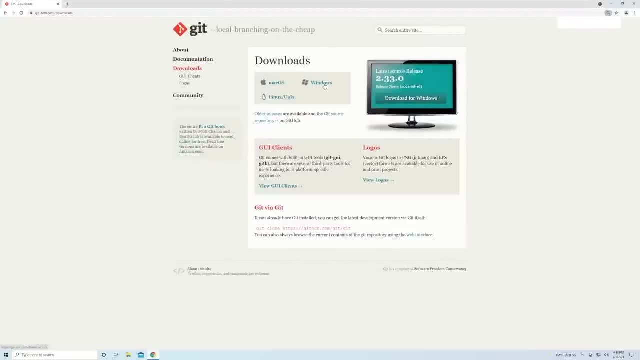 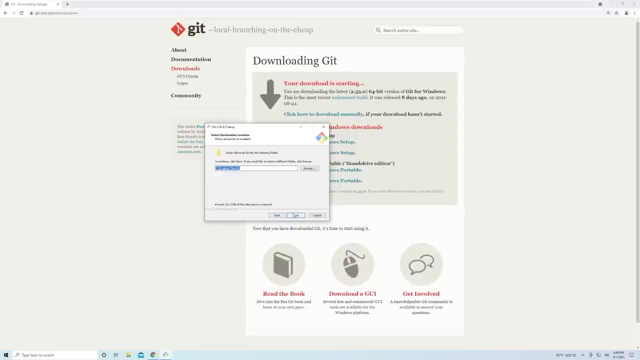 But regardless of your operating system, it's going to be a fairly similar procedure. So I'm going to select this, it's going to download that, All right, and then, when the wizard opens, go ahead and select next, Next, here, and you can leave everything default here as well, And here and here. 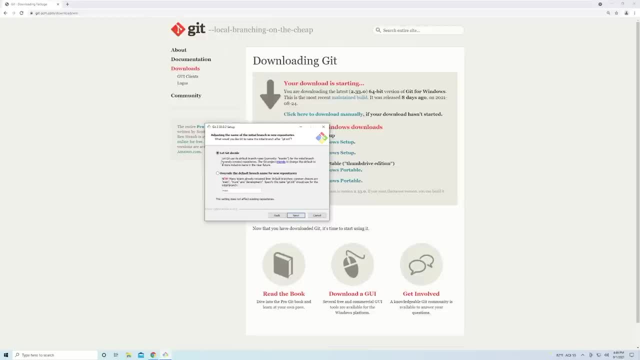 Now this is the one thing that we do have to change. So this is kind of a little bit of a nuisance at this point. But they used to call, like the main branch, the master branch, but I guess people are offended by that. 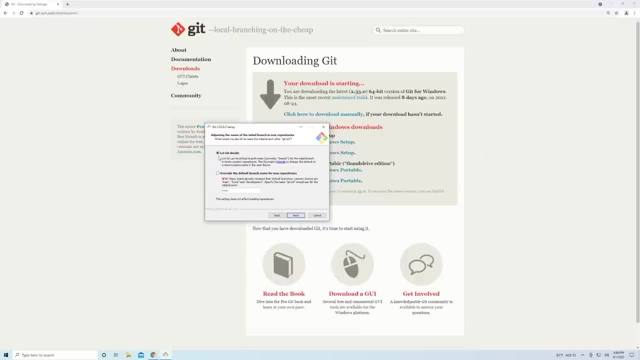 So now the new term for the main branch is main. So go ahead and override the default branch and just change that to main, Because when you work on GitHub they've already changed the default branch to be main, So we're going to want to do the same thing, So hit next And then you can leave everything as default, moving forward. There's a lot of windows to go through. 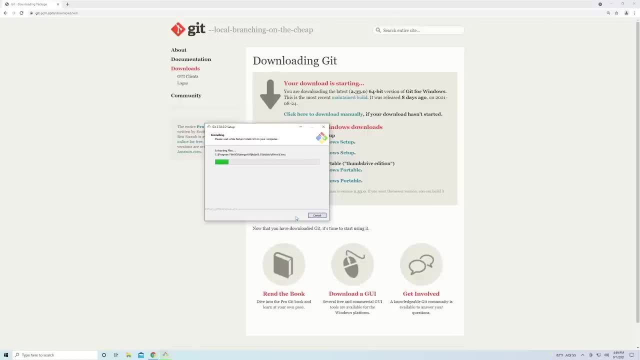 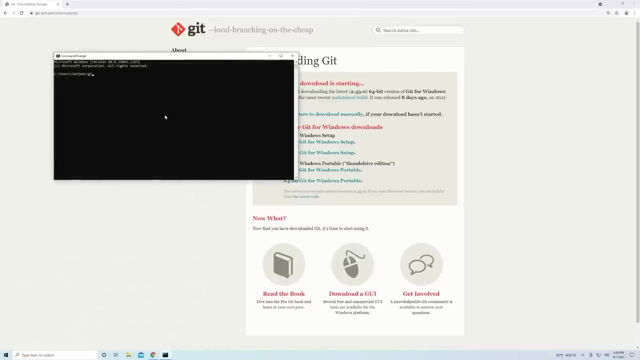 And then it's going to proceed to install git. All right, close that out. And then what you want to do is open up a new terminal And just type in git dash, dash, version, And if it spits that out, that means you've got git successfully installed. 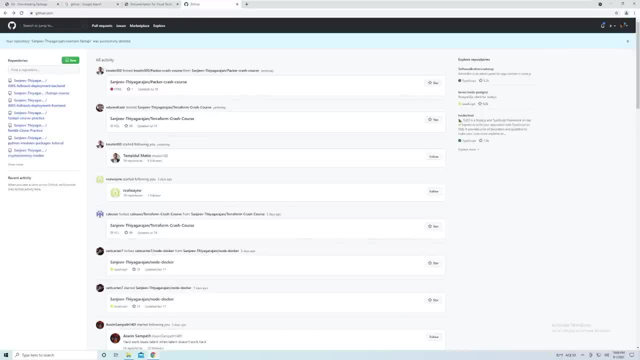 In this video we're going to set up a remote repository so we can store all of our code on GitHub, And so, if you don't already have a remote repository, you can store all of your code on GitHub. If you don't already have an account on GitHub, go to the main GitHub page, just go to githubcom and just click sign up and then follow those instructions And then, once that's done, just log in And you should see something similar to this, although you may not see an activity window if you just created a brand new account, because you won't have any repositories. 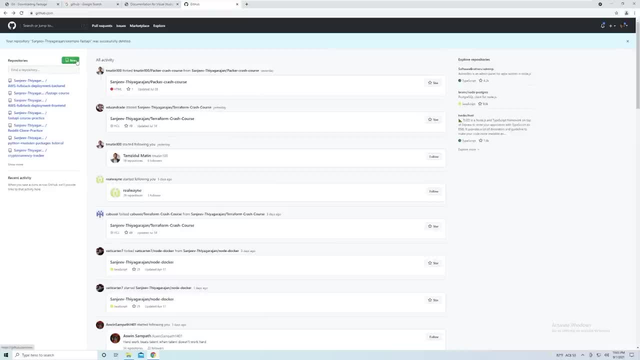 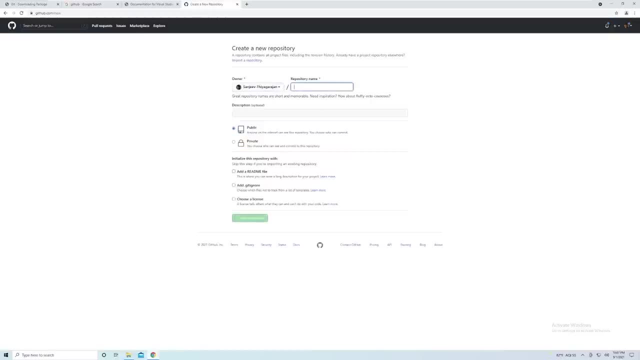 But just look for a new button, a button to create a new repository. You can also go up here, I believe, and select new repository. So I'll select new, And then we have to give our repository name. you can give it any name you want, I'm just going to give it a dummy name. So this is going to be example. 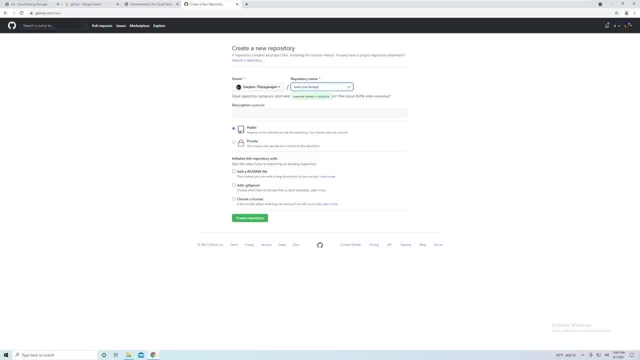 Fast API, but name it what after? whatever your project is Technically, I've already set up git for my project, just so I can track all the changes I've made throughout the course. But I want to make sure that I can walk you through this if you've never done it before. 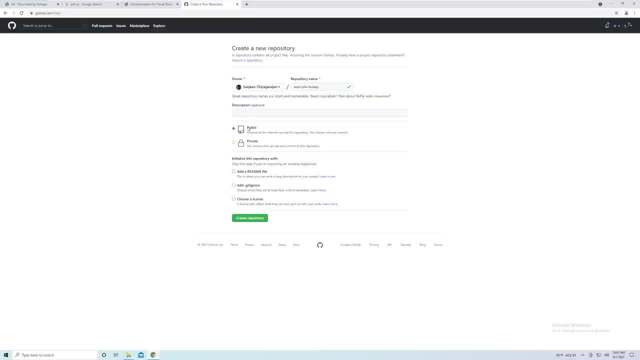 You can give it an optional description, And then you can choose whether or not a repository is public or private. If it's public, anybody can see it. If it's private, then only you can see it. we're going to keep it as public. Don't worry. if you decide to change it in the future, you can change it to private. 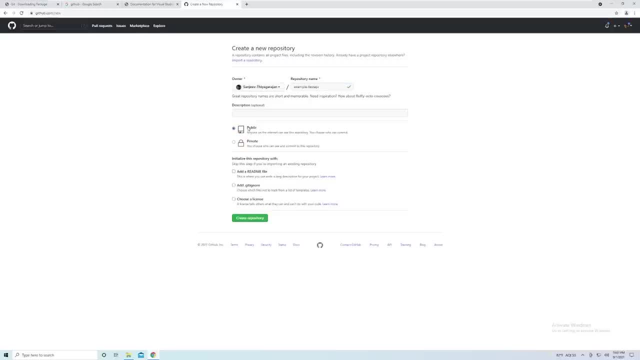 However, it does make a few things a little bit easier when it's public. So I'm going to leave this as public And then we're going to leave all these unchecked. they don't really matter And we'll select. create repository. 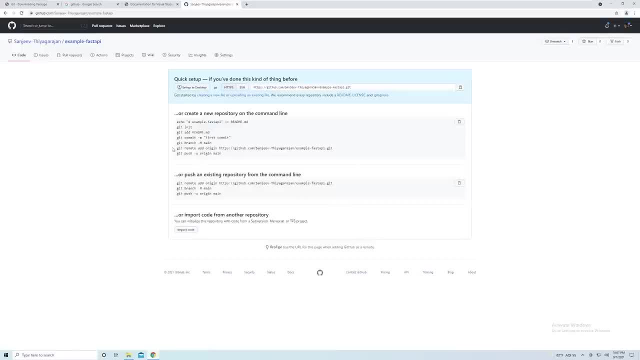 And then you'll see that it's going to give us a couple of steps to follow. So if we haven't already set up git for our project, these are the instructions we're going to follow, And if we've already set up git in our project folder, then we can follow these steps. 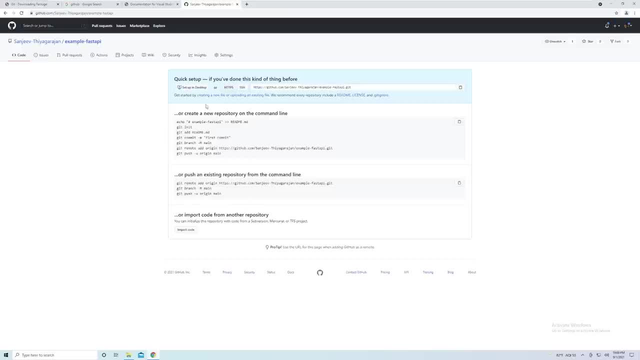 However, you know, we haven't set up git yet, So we're going to, for the most part, follow along here, But we're going to modify it just a little bit because we don't need to run some of these things together. 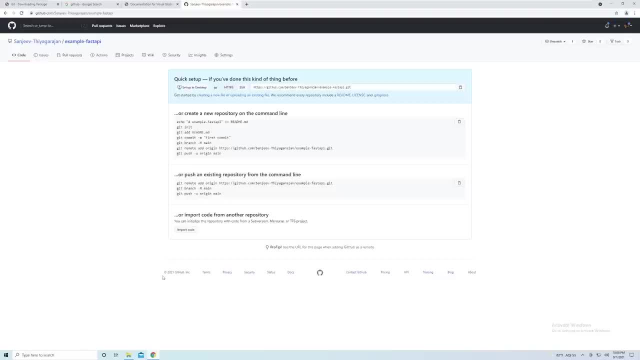 So we're going to hide it inside the console or use the essentially already set up git, and then we can select kun Get kept for logic use. So here's how we're going to do that a little bit, because we don't need to run some of these commands. So go ahead and open. 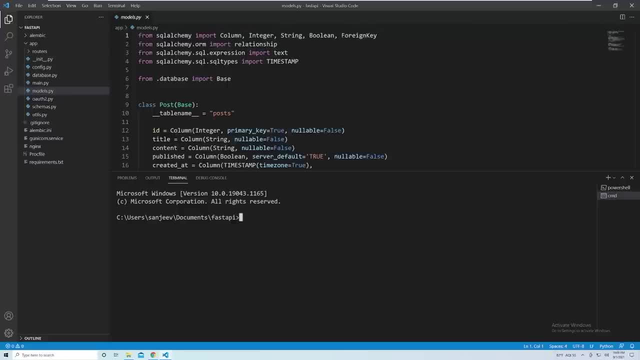 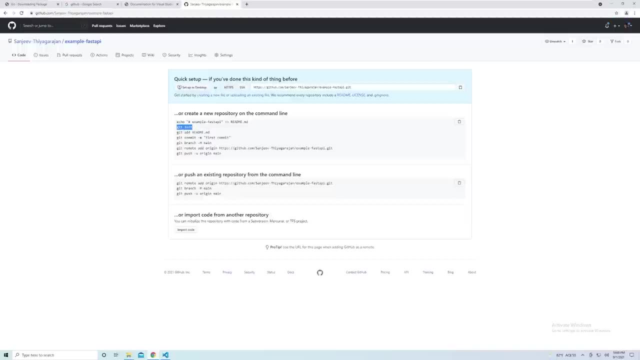 up your project in VS code like you normally do, Then open up your terminal And we're going to follow these steps, But we're going to ignore the first one. we don't need to read me for now, But we are going to do a git init which is going to initialize git. 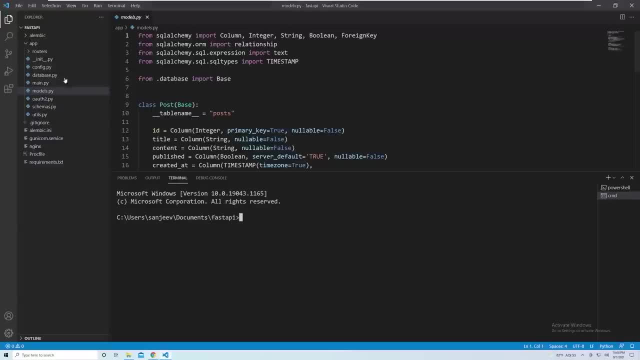 for our project, And so make sure you're at the root directory of your project. So, whatever this is called right here at the top, make sure that's where you're at And just do a git init. That's going to initialize git, And you may not see anything different about. 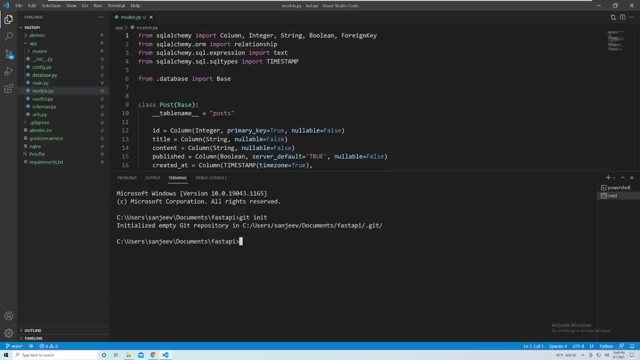 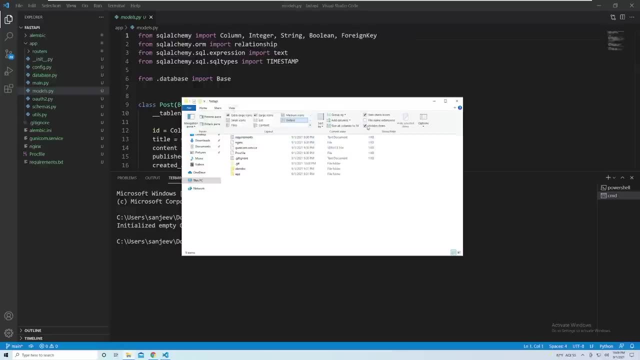 your folders. But I think it's because VS code actually hides the git folder. But when you actually did a git init, if you open up this, your project directory, and you click on View here and then make sure you select hidden items, you'll see that it created the. 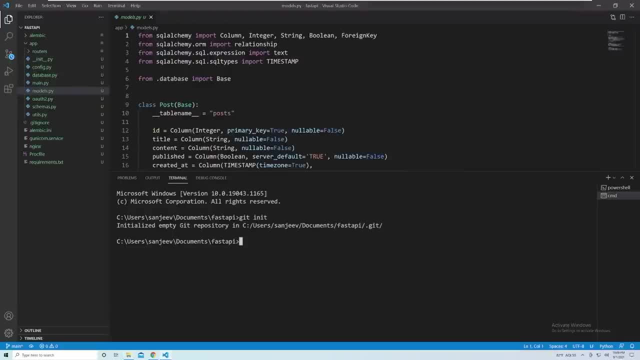 dot git folder. So this is where it stores all of the git information. Then we're going to skip this git add readme. Instead, what we're going to do is we're going to run git add, dash, dash all. So this is going to add all of the files that we have in our directory. 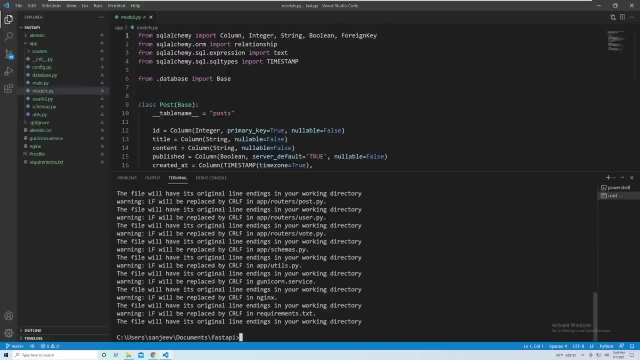 into git, Alright, and you'll get a couple of warnings potentially. don't worry about that, those won't create any issues. then we have to commit our changes. Anytime you add a file, you then have to commit it. So we'll say: git commit dash m. So the 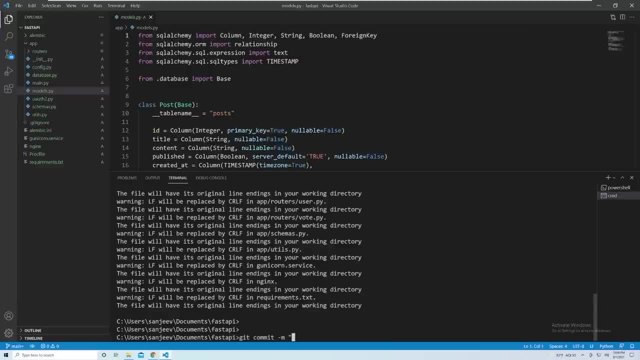 dash m means we're going to provide a message. So you usually give a message for each commit to kind of describe what changes you're making. So we're just going to call this initial commit Alright, and you'll see that we probably get an error if this is the first time you've. 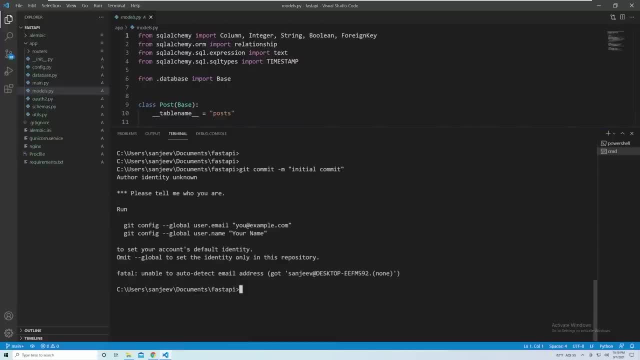 ever worked with git, And that's okay. It's just telling us: hey, we need to set up our user for our account on this machine. So we're just going to run this command right here And then we're just going to provide the email that we use to register for GitHub. 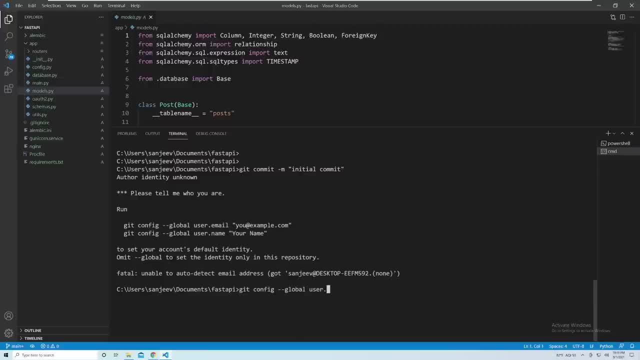 Also get config dash dash global user dot email. Alright, we set that. and then it's telling us to also set our name, So we'll do that as well. Then we're going to run that same command, the git commit. So if you just hit the up, 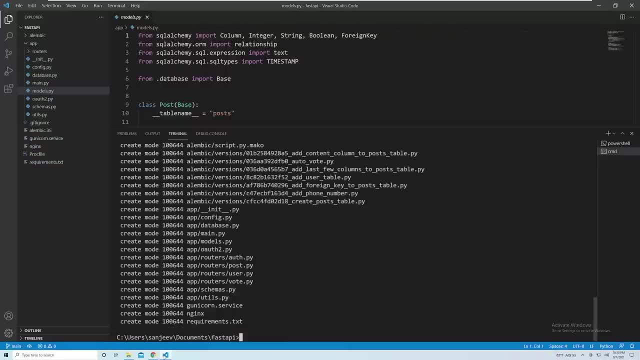 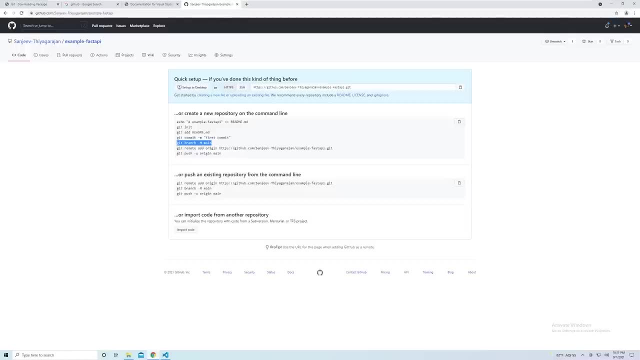 arrow a couple of times, you'll get to that. Alright, so we've committed those changes. then what we need to do is we need to set what our branches so here. this is just going to set our main branch to be called main, And so we can copy that, paste it into here. 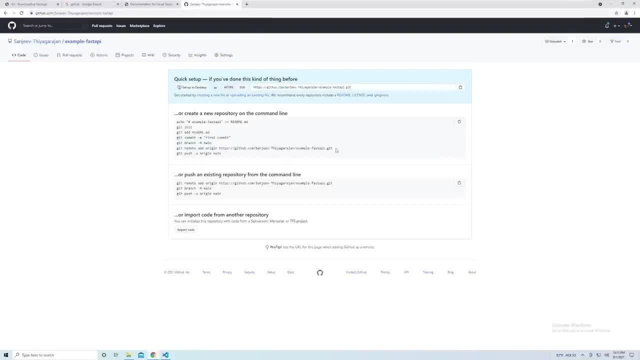 Then we have to set up a remote branch. So this is what's going to allow us to store all of our code On GitHub. So we're just saying, hey, listen, this is going to be the remote Git repository and we just provide a URL to it, And so that if you take a look at the URL, it's going. 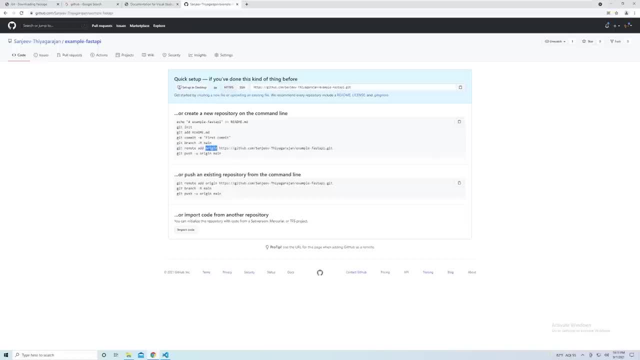 to match up with this, And in this case we're naming it origin. you can technically call it anything you want. We'll add that. And then, finally, we need to do a git push: dash u origin main, And so this means we're actually going to push all of our code up to GitHub, And you'll see. 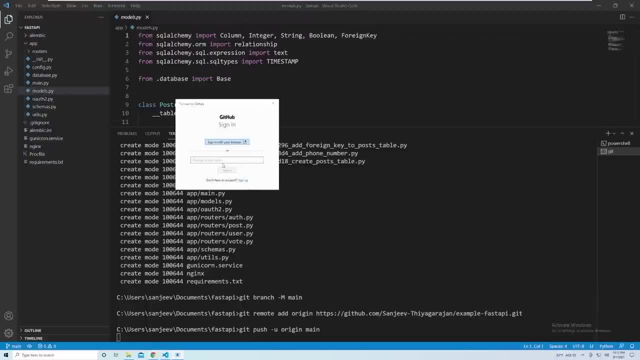 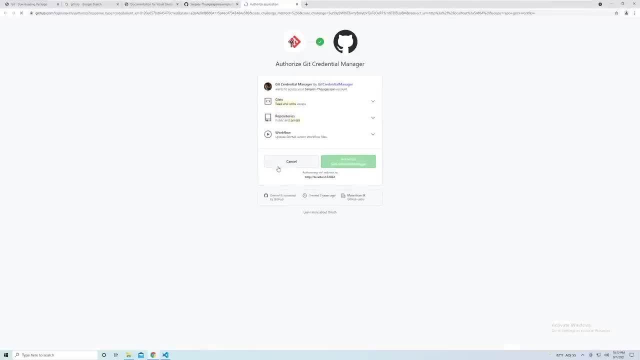 a pop up asking you to sign in, And there's a couple of things we can do. we can get a personal access token or we can sign in, Or we can sign in with our browser. I'm just going to sign in with our browser And we 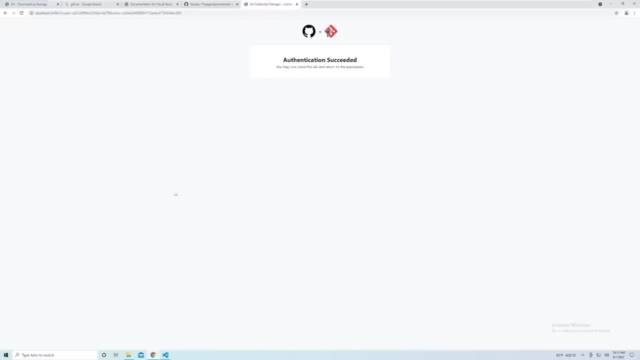 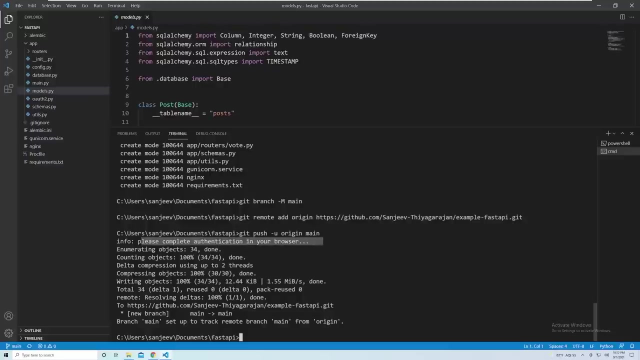 just like authorized right here And says it's succeeded, So we should be able to go back, And we can see that a couple things change. So it looks like that's our authentication, And then you can see that we're pushing all of this stuff up to GitHub, And so at this. 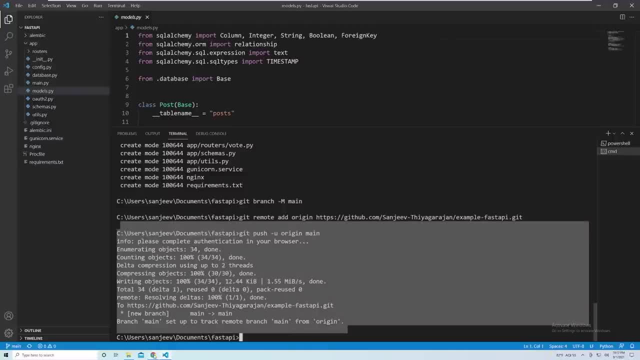 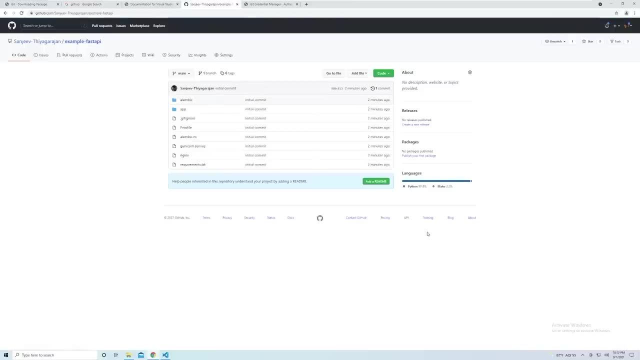 point you're pretty much done. all of your code is now stored in GitHub And we can just verify that by going back to this page and just like the name of the repository again And you'll see all of our core, all of our code, stored on GitHub now. So at this point, 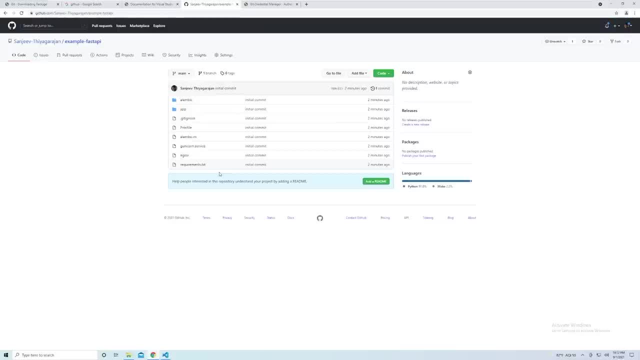 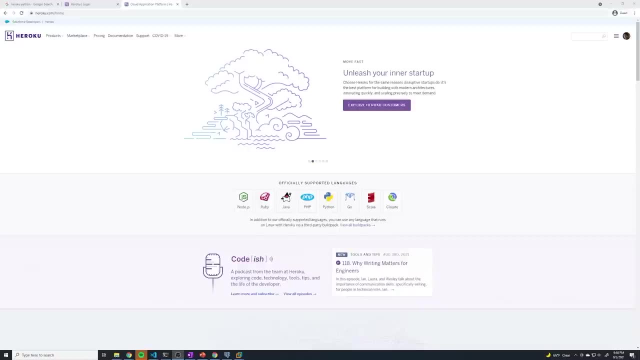 our repository is set up and we can move on to deploying our application. In this lesson, we're going to take a look at the first of two deployment methods that we're going to cover in this course. So what we're going to do is we're going to deploy our application. 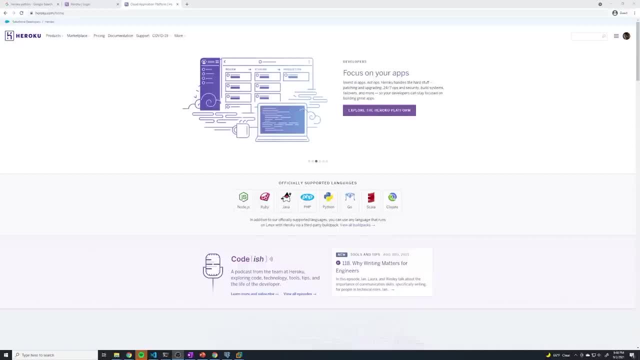 to a platform called her roku, And the reason I wanted to make sure to have this as one of the deployment methods was that her roku very generous, free tier, And so we can create an account for free And we can deploy our application absolutely for free, without having to pay a single dollar, And we don't even have 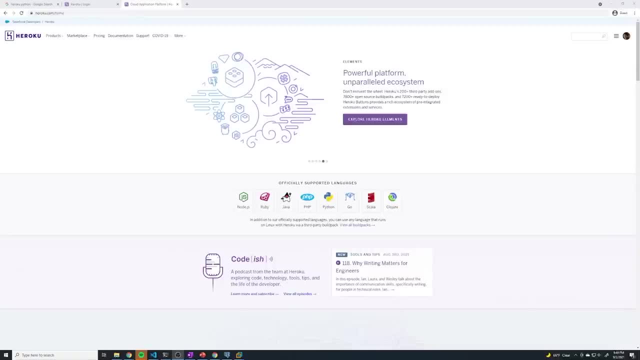 to provide our credit cards, And I wanted to make sure to add that just because I know for some of you guys that isn't exactly an option, And I wanted to make sure that you can still deploy your application and show off to your friends and family what you have created, And you'll see that. 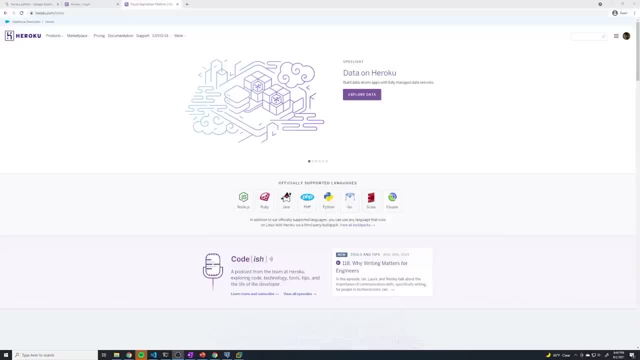 Heroku has made it very easy to deploy your application And it's very easy to push out changes to your application. It's a fantastic platform And I think you guys will learn a lot on how to actually deploy an application by making use of a platform like Heroku. 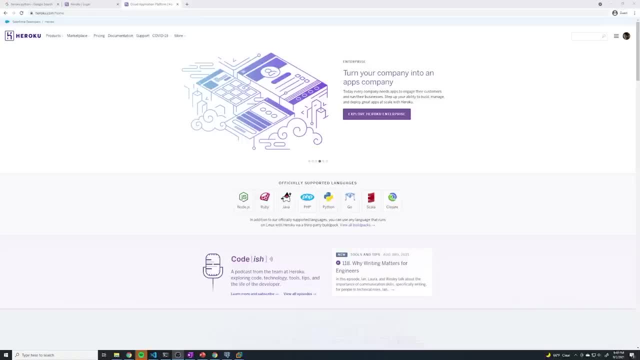 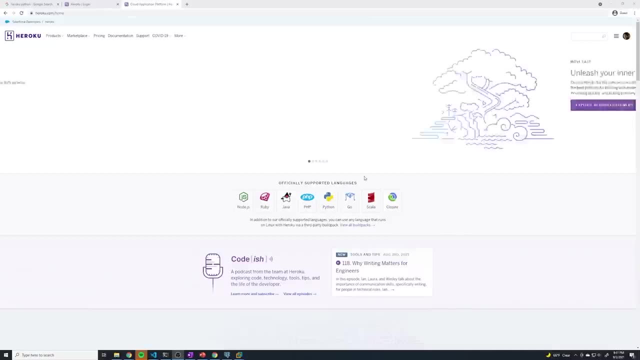 So we'll take a look at how we can, you know, make use of Heroku, learn about the Heroku CLI so that we can push our application to the platform and, ultimately, have anyone be able to access our API. Heroku has a lot of really good tutorials on how to deploy applications on their 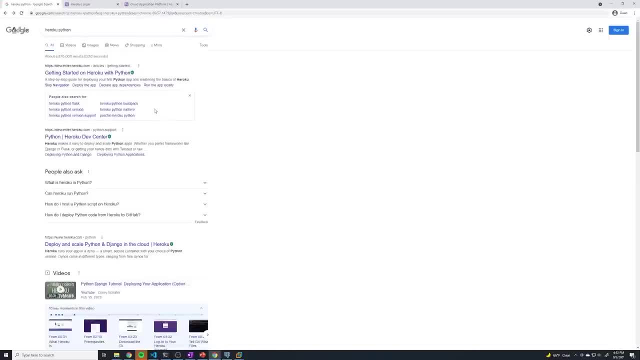 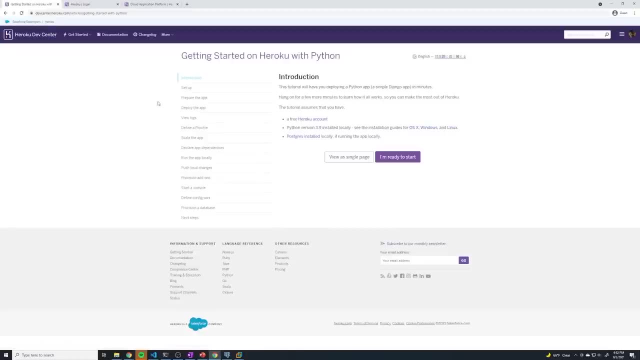 platforms, And they've got one for Python as well. So if we go to Google, just search for Heroku Python And the first result is going to be their tutorial. it's going to walk us step by step on how to actually deploy our application. But before we do that, there's a couple of things that we 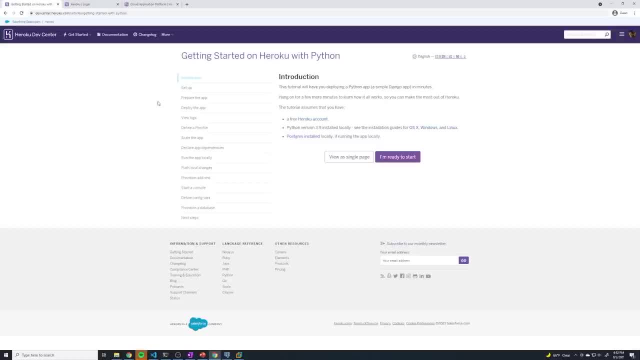 have to do? First of all, go ahead and create an account on Heroku If you don't, if you haven't already done so, it's completely free, So just provide your email and so on. Then there's two other requirements we have to have get installed on our machine, which we've already done, And 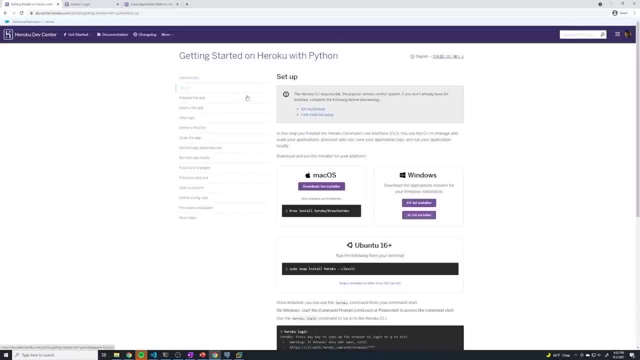 then finally, we have to install Heroku itself. So if you go to the setup section right here, you're going to see the installers for all of the different operating systems they support. So just select whichever operating system you have and get the Heroku CLI installed on your machine. And after you get it installed, 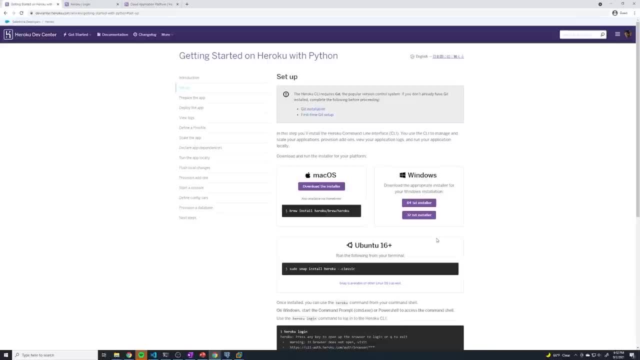 usually you have to close out any of your pre existing terminals and reopen them to actually be able to access the Heroku command. If you have VS code, a lot of times I've had to just close out VS code altogether, not just close the terminals but actually close out the entire. 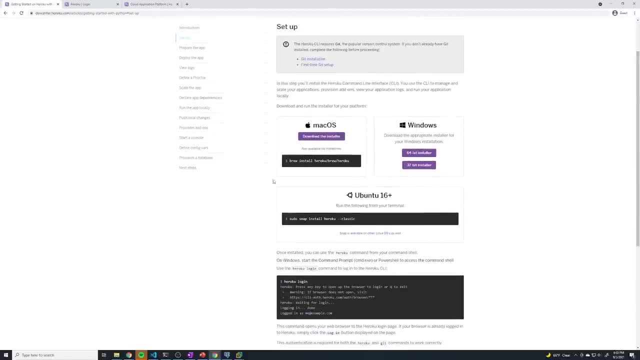 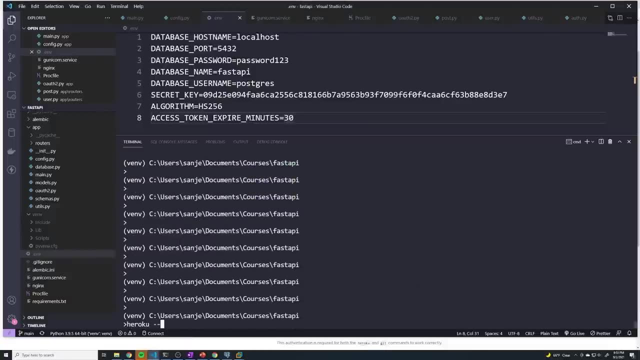 application and then open it back up. But after you've done that, if you want to verify if Heroku was successfully installed, just go to Heroku, And then you're going to have to close out the version. So go to your terminal and just type in Heroku, dash, dash version, And if it spits out a 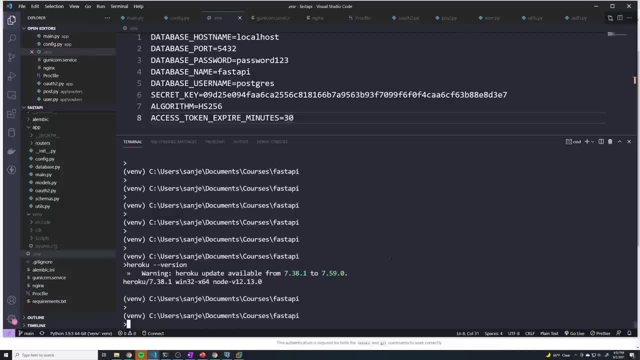 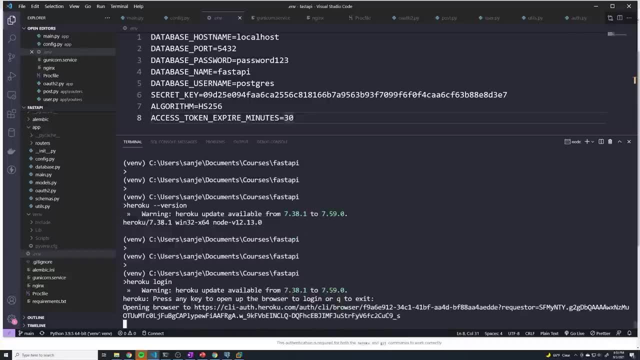 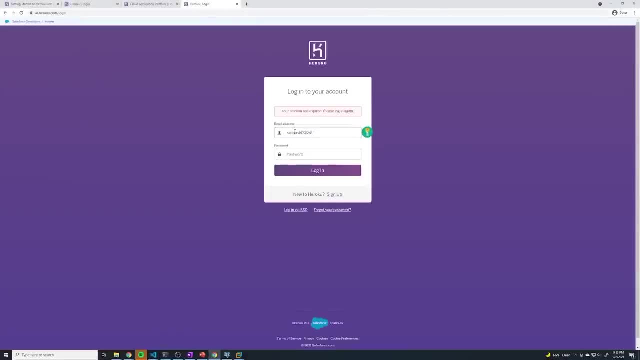 version. that means Heroku has been successfully installed, And after it's been installed we want to log in. So we do Heroku login And then you just press any key right here And it's going to open up your web browser. you can just log in and then provide your credentials, All right. 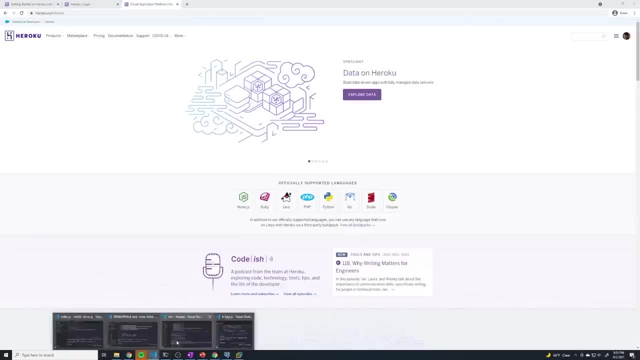 and then, once you're logged in, you can just close it up, And then you're going to have to close it up. We're going to close out this window. go back to our code And you can see. logging in is done And. 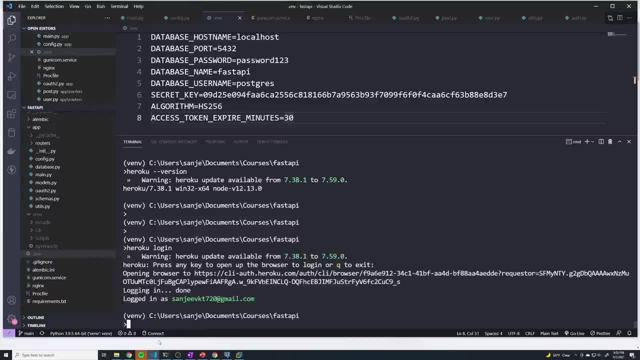 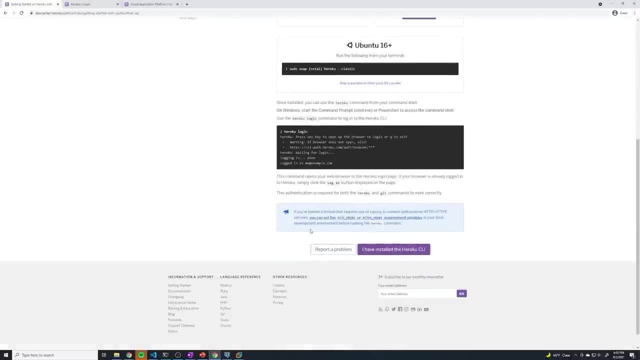 we've logged in And then that's my specific account right there. All right, And once that's done, we're going to go back to the tutorial And we're just going to kind of follow along. So if you go to prepare the app, you can ignore this. So they give you like a demo application to kind. 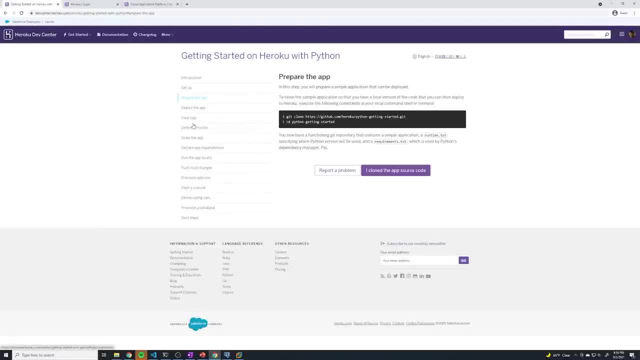 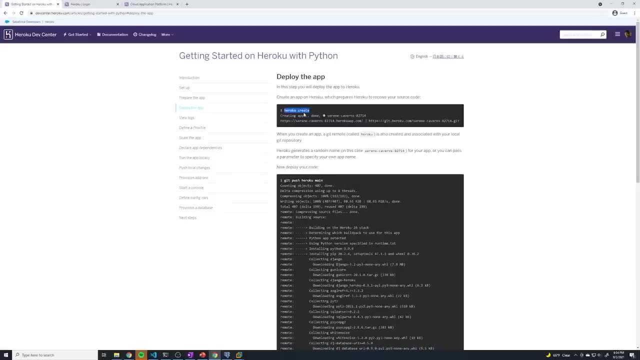 of follow through the tutorial, but we already have our own app, So we don't need to worry about that. If we go to deploy the app, we have to run this command: Heroku Create. So we have to create an app within our Heroku account. So let's run that command. 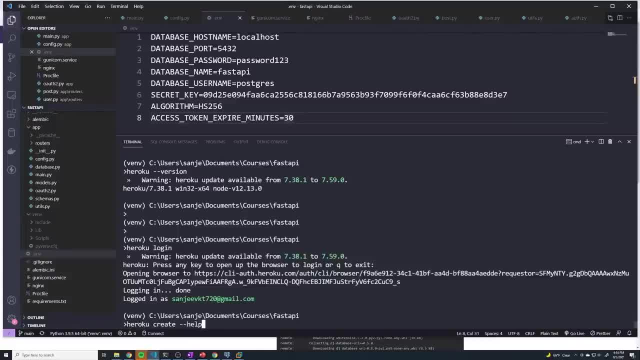 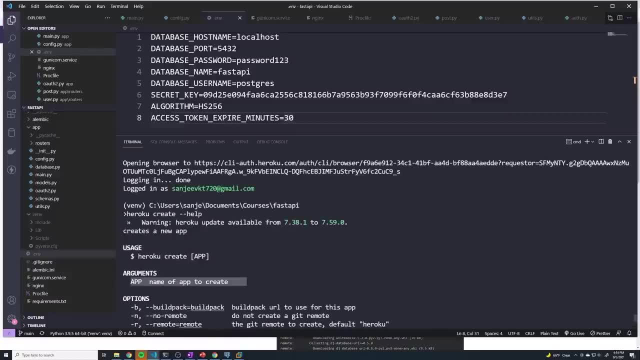 But before we run that, I'm going to do a Heroku create, dash, dash help, And we can see that one of the arguments is going to be the name of the app we want to create, And so if you don't provide a name, Heroku just gives you a random name. But I always like to. 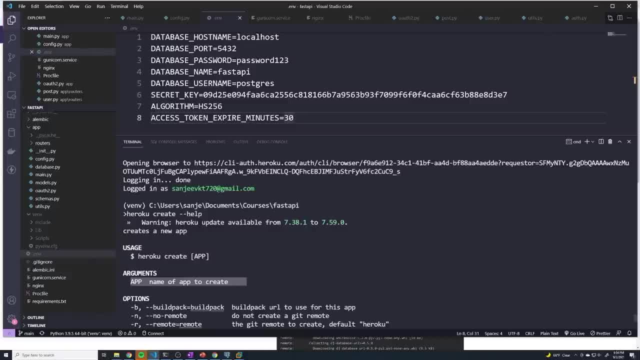 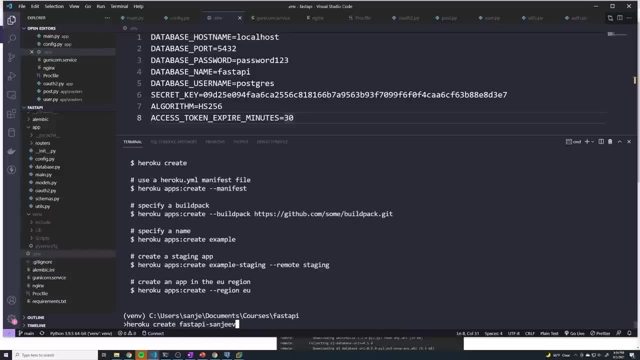 use a more familiar name. So I know that what app, which app covers which one of my applications, And so I'm going to call this fast API Sanjeev And keep in mind these app names are global, So if I deploy my app as fast API dash. 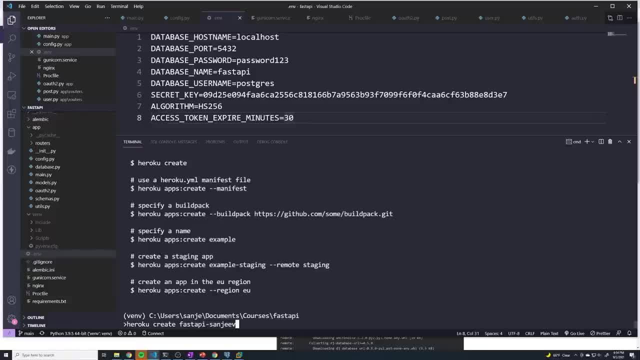 Sanjeev, you will not be able to create an app with the same exact name, And that's because, to actually access our application once deployed, the URL is going to be the specific app name embedded in there, So it has to be globally unique. So if it says your, your app name is already taken, then 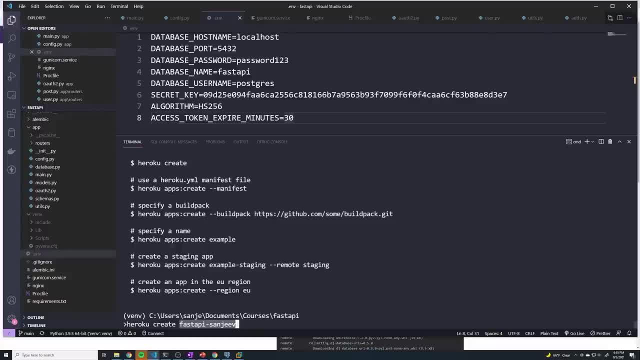 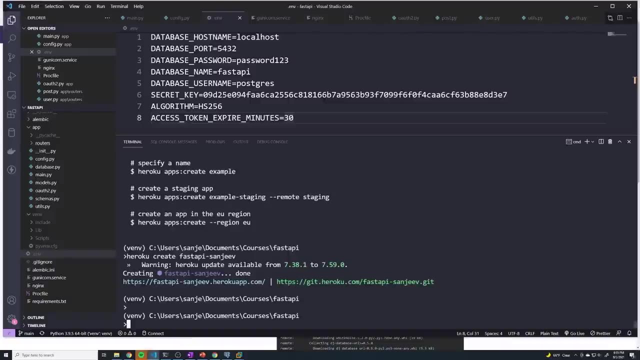 just try a different one, maybe add a couple of numbers at the end. it doesn't really matter what the name is: Sanjeev. All right, and once we've created our app, the next thing that we have to do is: well, actually, before we even do that, I want to show you guys what it actually did. 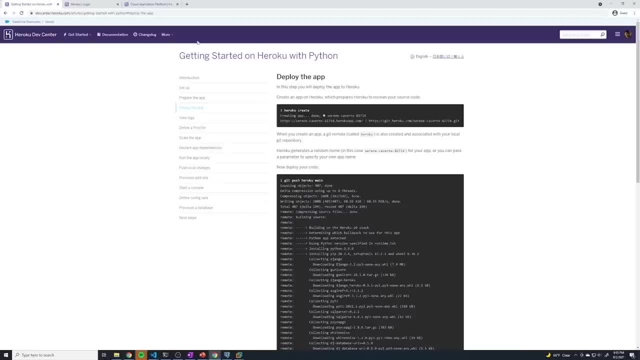 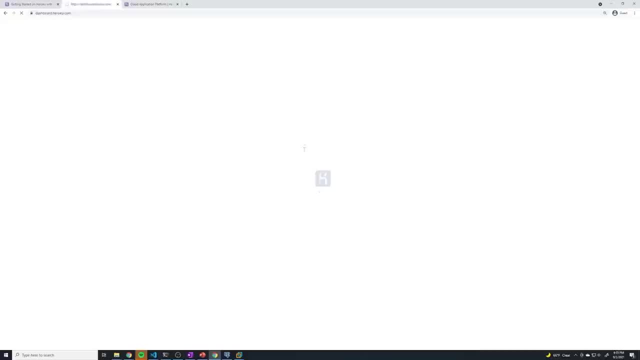 So there's a couple things that happened behind the scenes, And the first thing is if we actually log into our account- I'm going to log in right here- We're going to see our dashboard, So in the dashboard you can see the application that. 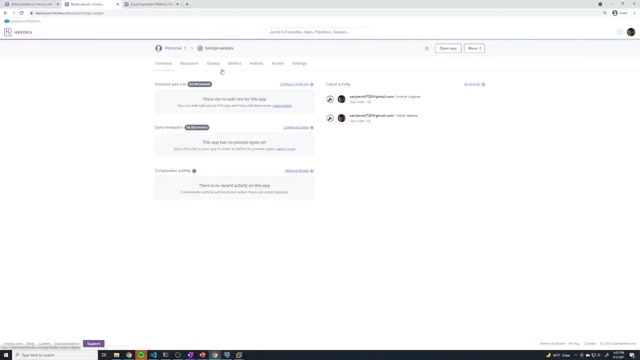 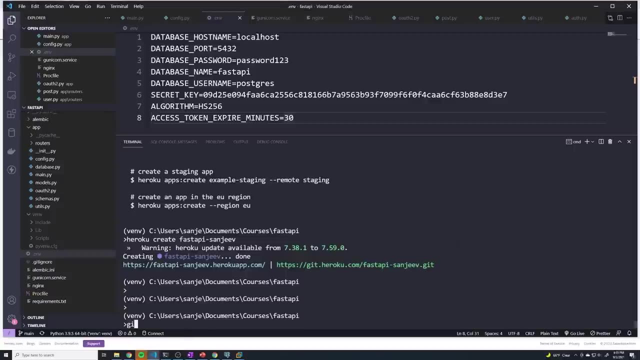 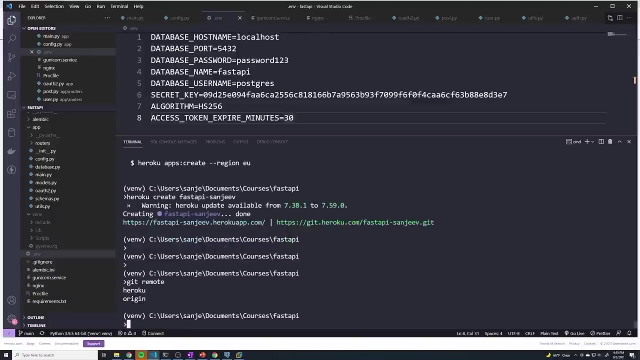 we just created. Right now there's nothing interesting. nothing's been set up with it, So we can actually see anything. But the second thing that it also did was, if I type in get remote, this is going to show all of the remote remotes that have been set up for our get And we can see. 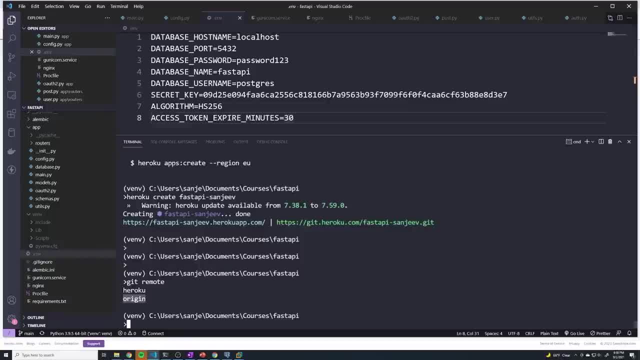 there's two now. So there's origin, which is the one we set up originally, and that's GitHub ultimately. but Heroku added a second one, And so this is ultimately how we deploy our application, because instead of doing a git push origin main to push it out to GitHub, we can just do git push. 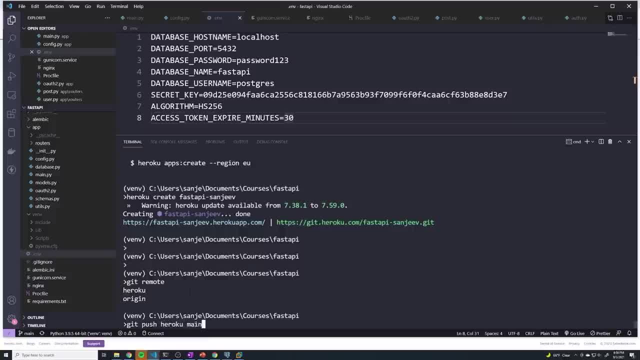 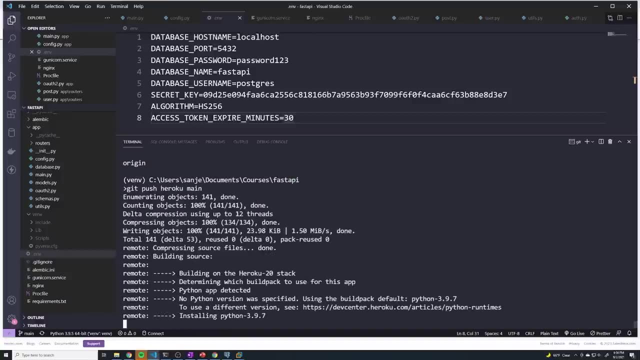 Heroku, Heroku main, And that's going to push out our code to the Heroku platform and then it will then create an instance for our application. So let's go ahead and do that. we're going to do a git push Heroku main And this is going to take a little bit of a while because it's got to, you know. 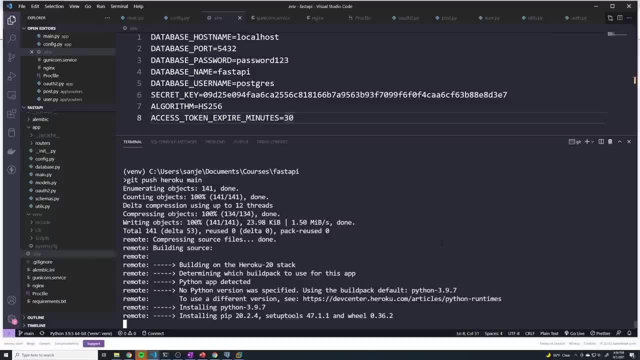 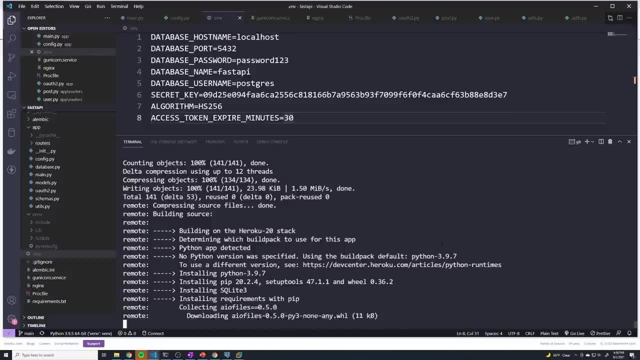 set up Python. it's got to do a few other things. it's got to install all of our dependencies before it can actually get our app up and running. So I'm going to pause this video and then I'll touch base with you guys once that's complete. 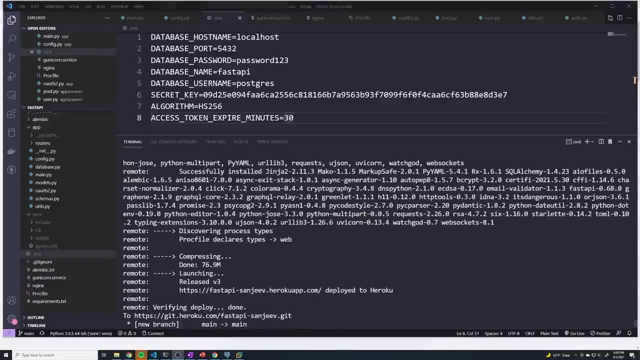 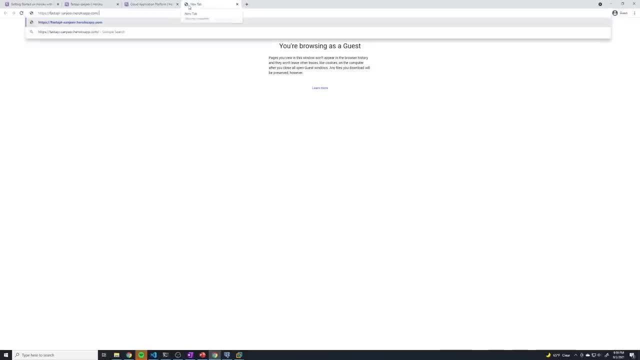 Alright, so our application has successfully been deployed And you'll see that in the logs, Heroku actually gives us the URL of our application. So I'm going to copy this URL and we're going to just open this up in the browser. And if you let this run long enough, 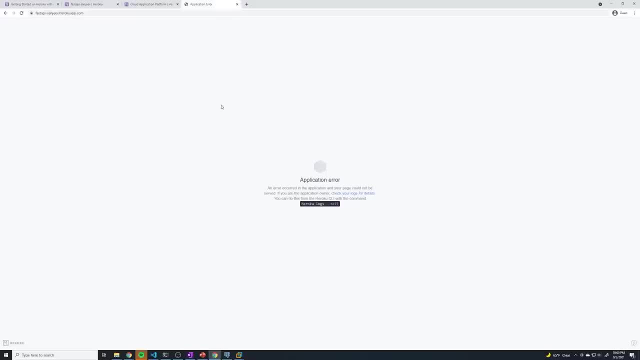 you're eventually going to see an error. So it looks like something in our application is broken, And this is to be expected, because there's still a few more things that we have to do to actually get this set up. Because, if you take a look at what we've done, we pushed out our code to Heroku. 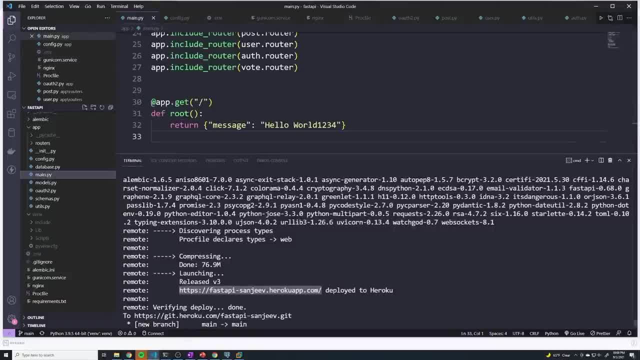 right, But Heroku has no idea. Heroku has no idea how to actually start our application. That you know what is the command? it doesn't. it just knows that this is a Python app, but it doesn't know what it is. It doesn't. 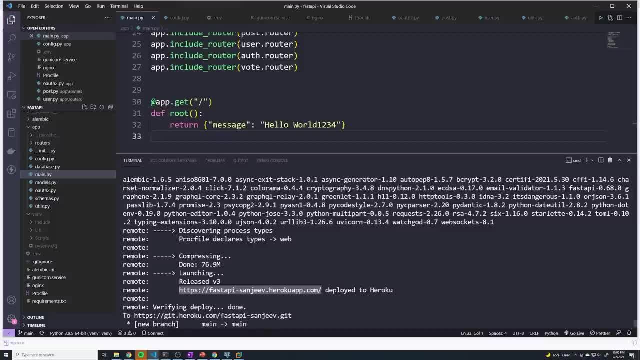 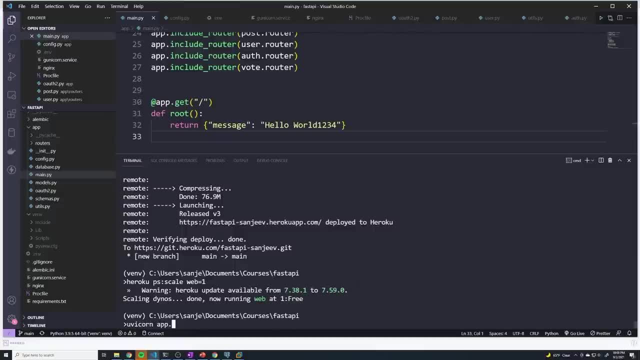 know that it's a fast API app. it doesn't know that we're trying to build out an API. it has no idea. And when we deploy to our development environment, we ran UV corn and then you know, app dot main and then app Right, but we haven't given that command to. 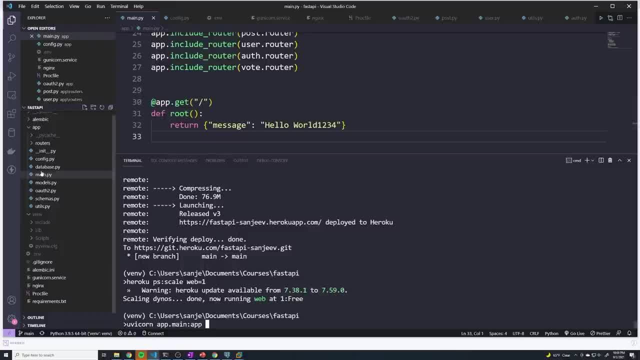 Heroku. how does it have any idea that our code is in main dot, p, y And that within the mainpy file we have our app instance stored in a variable called app? it has no idea. So what we have to do is: 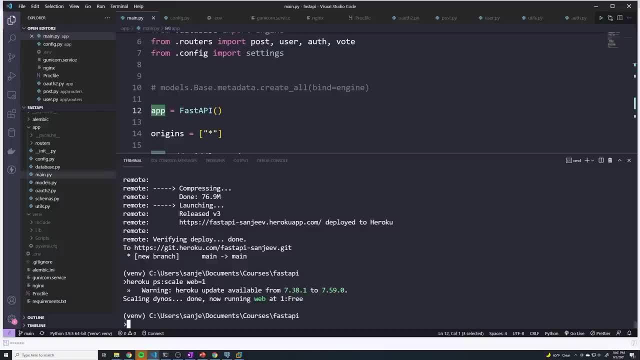 we actually have to create a file that's going to tell Heroku what is the exact command that we want to run. So inside your root directory. so just kind of collapse all the folders inside your root directory. So just right click here, create a new file, create a file called a proc file. So 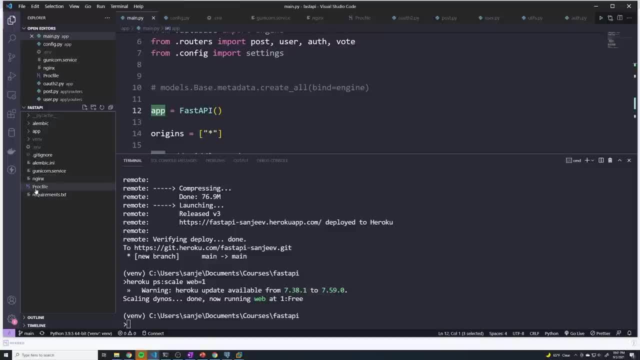 I've already got this in here. it's going to be in the GitHub repo So you can take a look at it and make sure you capitalize the P. And actually, if you take a look at the tutorial and we go to, 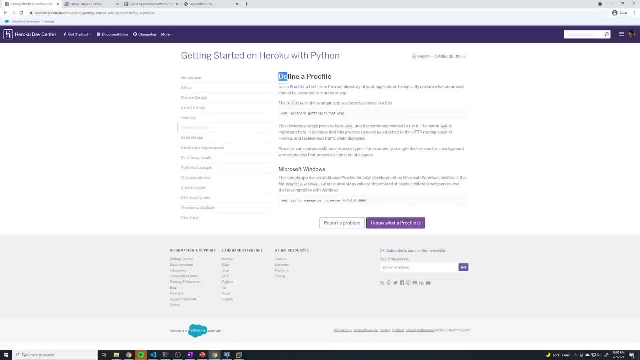 the next one, which is define a proc file. this is going to just explain what the proc file is, But the proc file just just tells Heroku what is the command that we need to start our application, And so here we give it a process type. So the, since this is a web application, that's going to 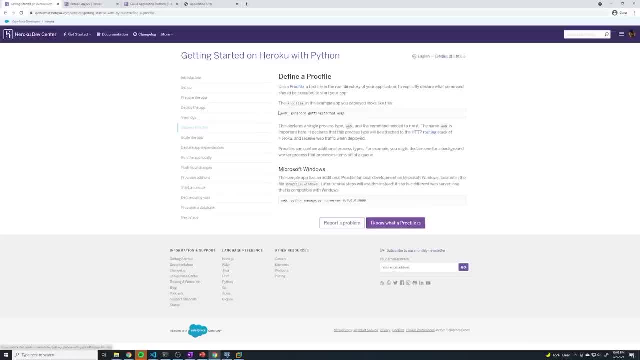 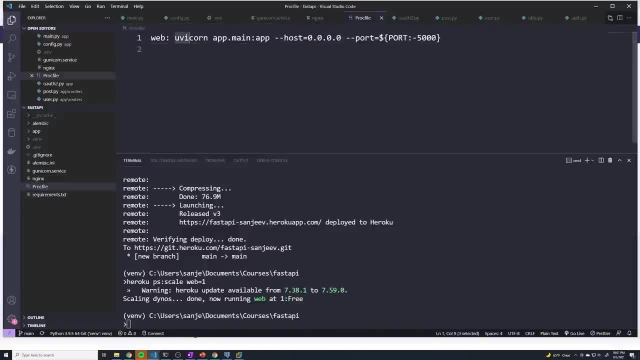 be responding to, you know, web requests. we want to use the word web and then we specify the exact command that we need to run, And so in my proc file a couple of things have been set up. So we run the command UV corn app dot main and then app, like we've done before. we're not going to pass in. 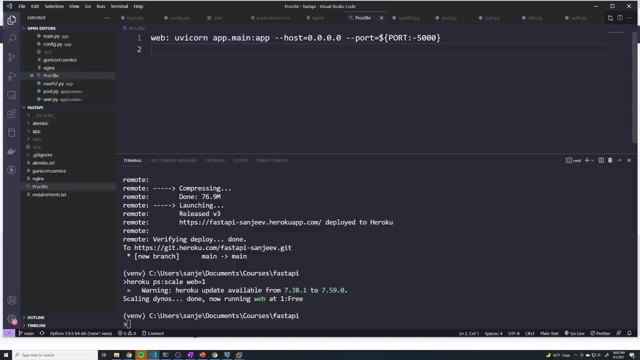 the dash dash reload flag. So we're going to pass in the dash dash reload flag And then we're going to pass in the port flag, because this is production. we don't want it to automatically reload on changes, because there should be no changes. we do have to provide the host IP. So this is just. 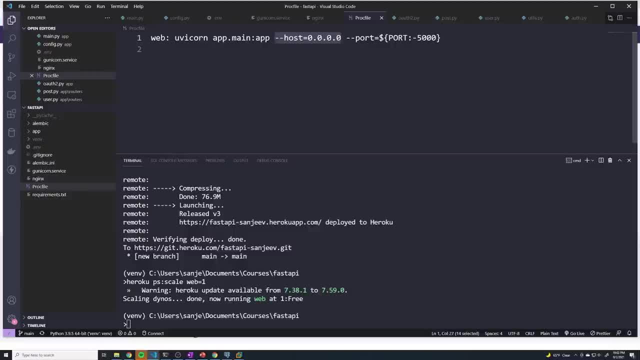 saying that, hey, we should be able to respond to request to any IP. So, whatever IP Heroku gives us, this is going to accept it. then the next flag is going to be the port flag. So what port should we run this on? If we don't provide a port flag, then it's going to default to port 8000.. Like it always. 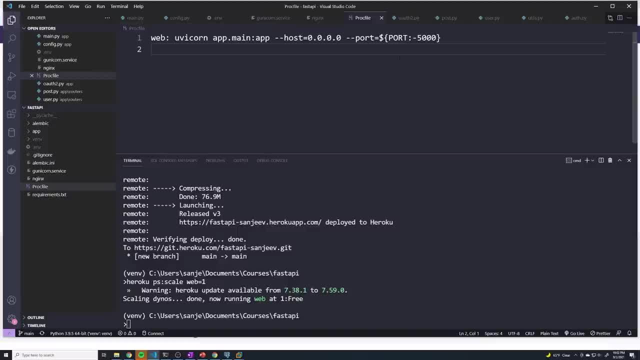 has. However, the thing about Heroku is that they're actually going to provide us a port, So we don't know what this port is going to provide us a port. So we don't know what this port is going to is ahead of time. So we have to be able to accept this port regardless of what it is, And so it's. 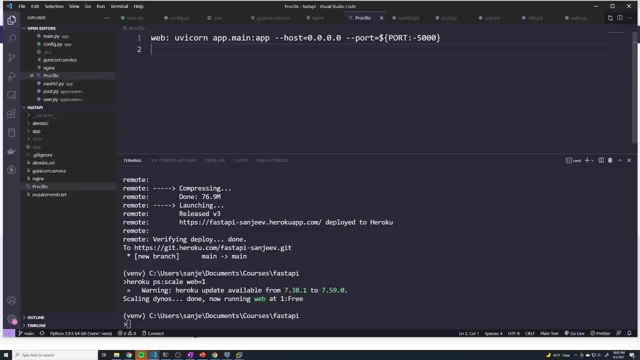 actually going to pass this down as an environment variable. So anytime you want to accept an environment variable or reference one, you can just say dollar and then curly braces. So we're really just saying we want to take whatever value Heroku gives us with the environment variable of. 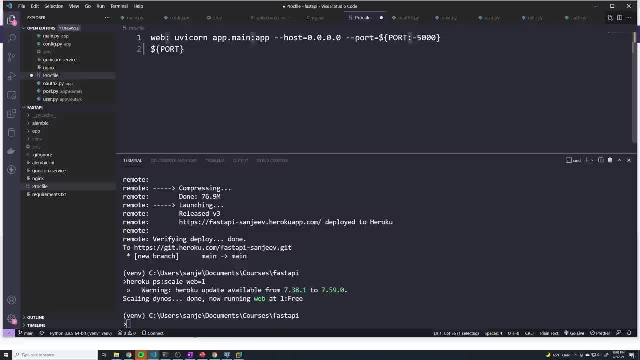 port and we want to assign it here, And then this is just giving it a default value of 5000.. If they don't provide one, however, Heroku will always provide a support, So I don't think we even need that. 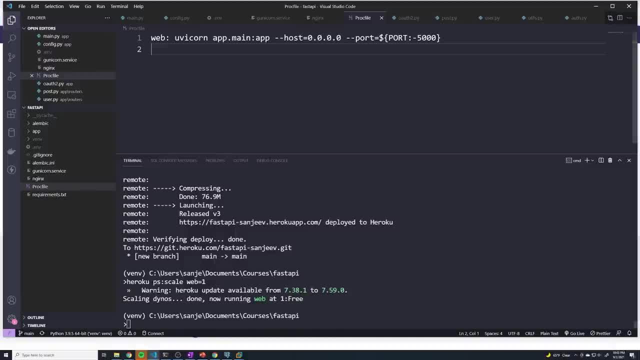 So after you make this file, you're then going to have to push out these changes to get once again, And since I already had this file, there's nothing to change in my gets or nothing will get pushed out. So I'm just going to just change some random code. I'm going to delete this 1234 here. 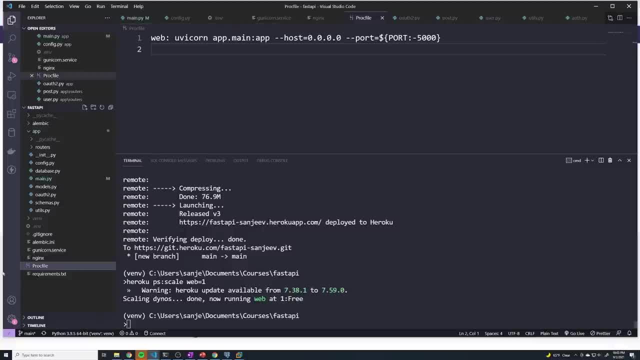 So that I can at least have some changes in my code. you guys will already have changes in your code because you added the new file, So then go ahead and do a git: add dash, dash also. that's going to add all the changes. we're going to do a commit. 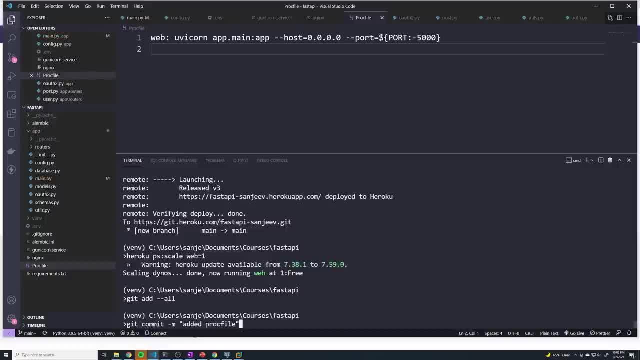 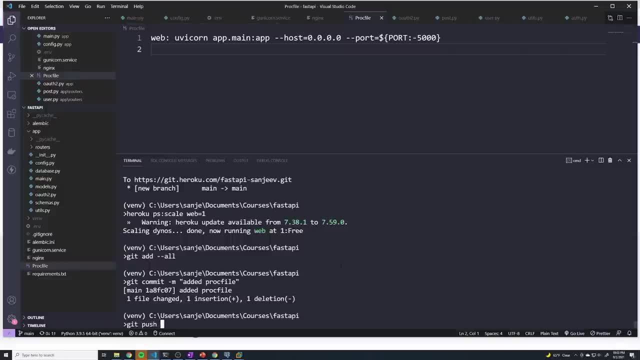 And we'll give it a message of added proc file. And then we do a git push. And then what do we push to? Well, first of all, you know, moving forward, we want to make sure that this is stored in GitHub. So 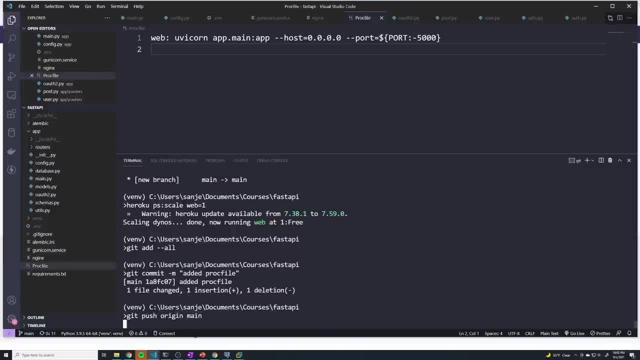 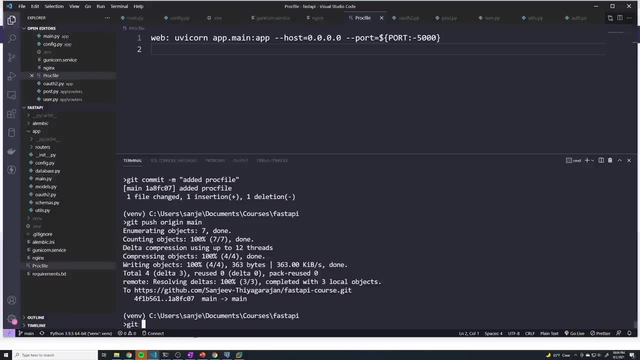 let's do a git push Origin main. this is going to push it to GitHub. And then now we want to actually push out these changes to Heroku so that we can actually get our application up and running. So we'll do a git push Heroku main. 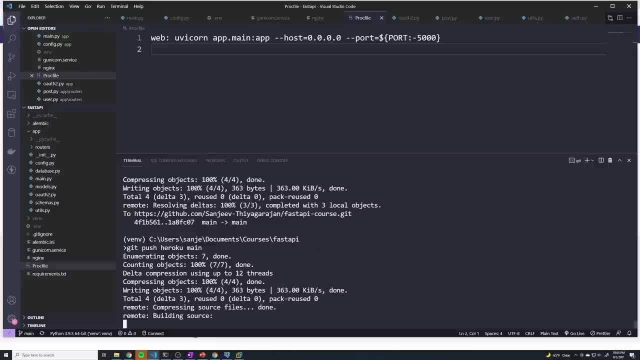 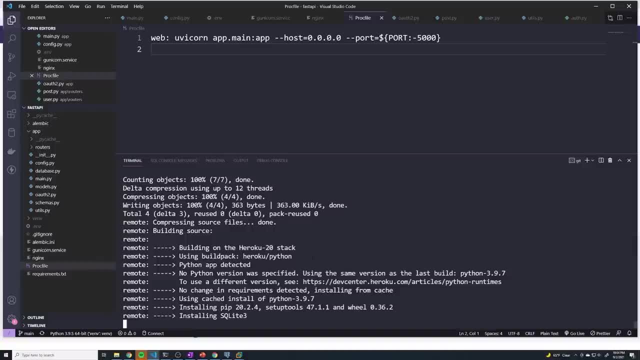 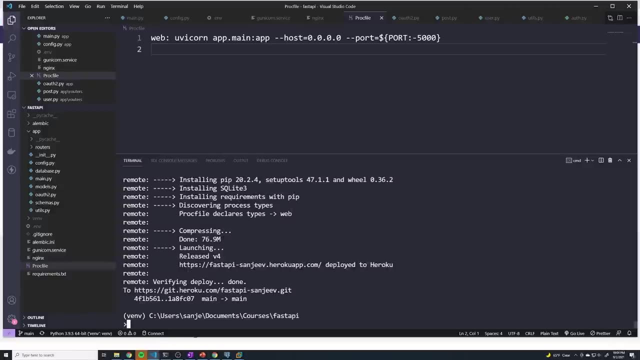 Again expect devices And once again we have to kind of wait through this entire process. Okay, so it's now finished. Once again, we're gonna go back to the URL it's deployed at And I'm just gonna do a refresh to see if we fixed our issue And the fact that it's still spinning. 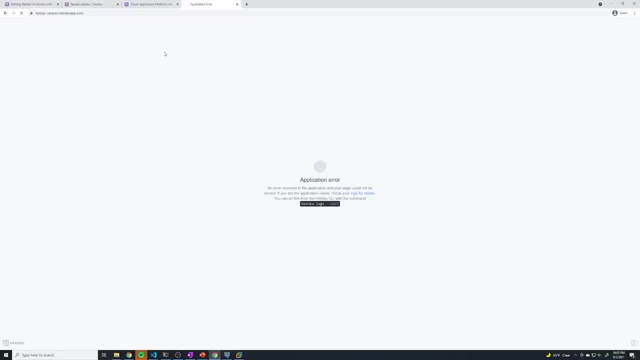 for this long most likely means that we did not fix our issue, But I already know the exact office credentials we used that we deployed, So let's go back there reason why this is, And so we will take a look at exactly what is causing our application to. 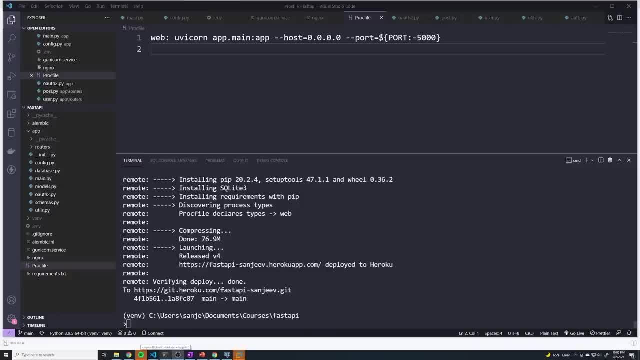 not successfully get deployed in the next lesson. Anytime your application isn't working, on Heroku, his platform, they have a really easy way of accessing logs. So we can say Heroku logs and I'm just going to do a dash, dash help, just to see what options we have. 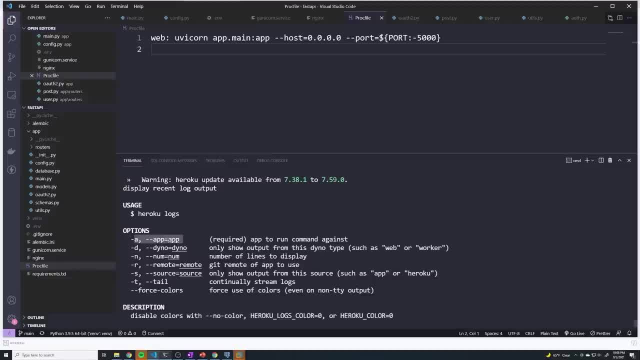 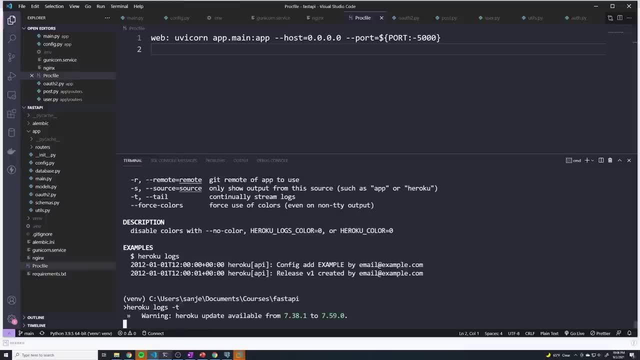 And so here we could specify the app or we can just dump the logs for all of our apps. But what I'm gonna do is I'm going to pass in the dash T flag so we can tail the logs as things happen. So if I do a dash T And we scroll up, you can see that we've got a couple of different. 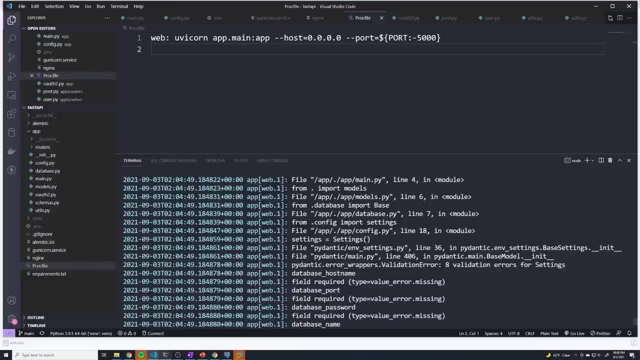 errors, And so it looks like there's some issues with settings, which, you know, is the, the pydantic model that we've set up for retrieving our environment variables, And it's saying that there's a couple of validation errors for our settings model, And it says that, hey look. 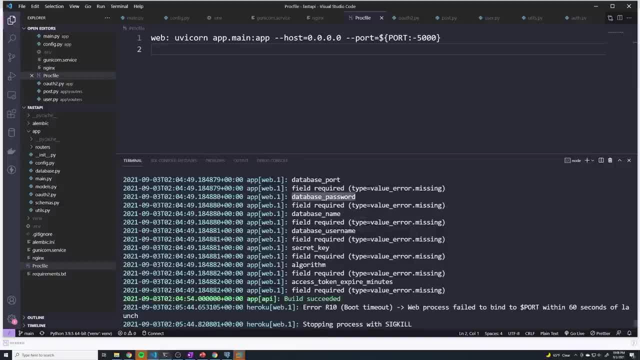 we don't have a database hostname, we don't have a database port password or any of the other information, So we're going to pass in the dash T flag so we can tail the logs as things happen. So there's some issue with our environment variables. And this makes sense Because in 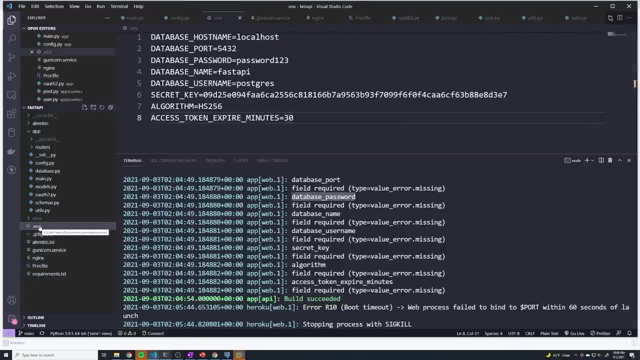 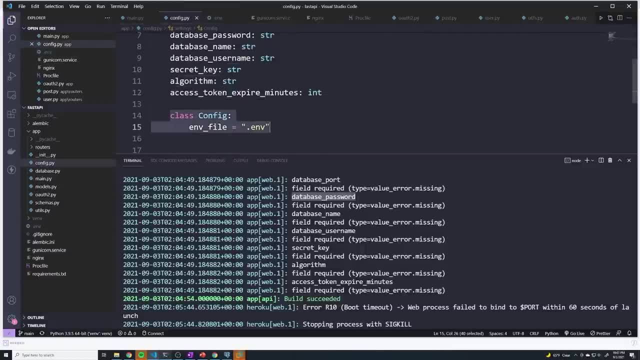 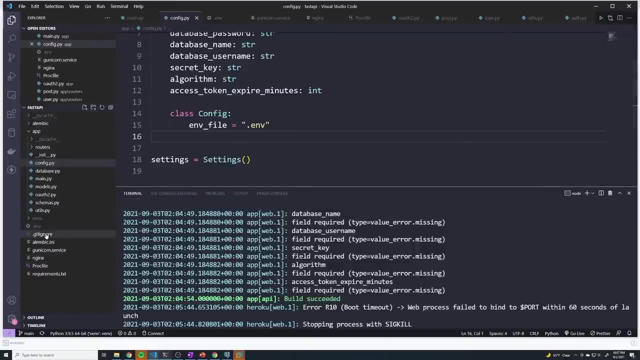 development. we use our dot env file to provide all of the environment variables into that settings model right here And we pass that by specifying the env file. However, we did not check our env file into git. Remember, in git We use the git ignore file to make sure we excluded. 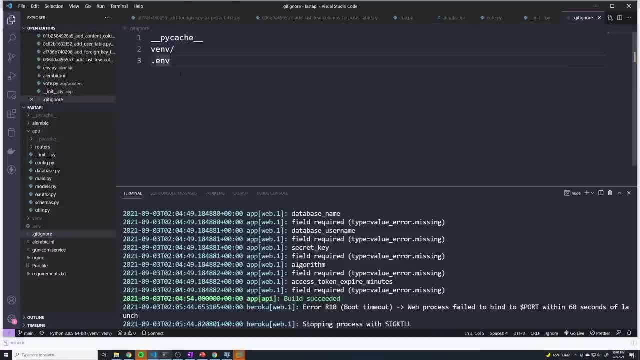 that, because we don't want to actually check that into git. So how does Heroku know what all of our environment variables should be? Well, they have the and so we actually have to add those environment variables either through the command line or through the dashboard. But 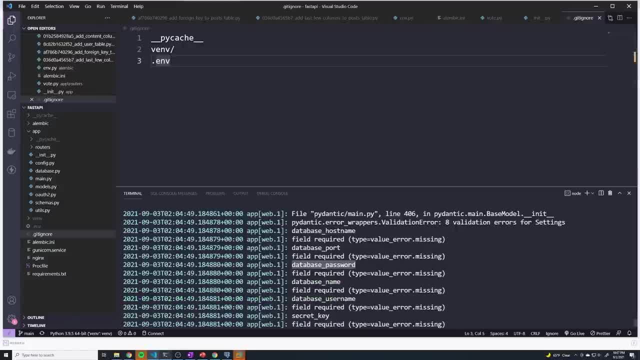 before we can do that, we need to actually get a Postgres database, Because right now we don't have a Postgres database. So what would we even provide for database hostname and port and password and things like that if we don't have one? So let's create one. And, once again, Heroku provides us. 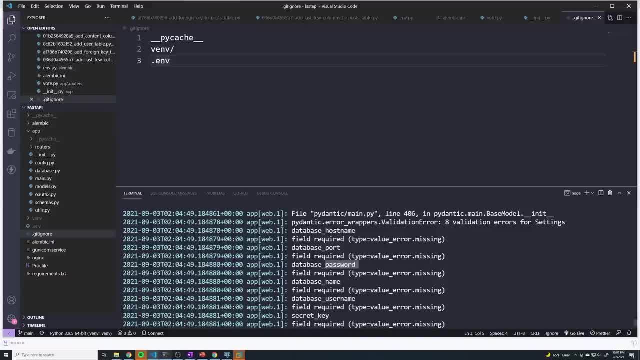 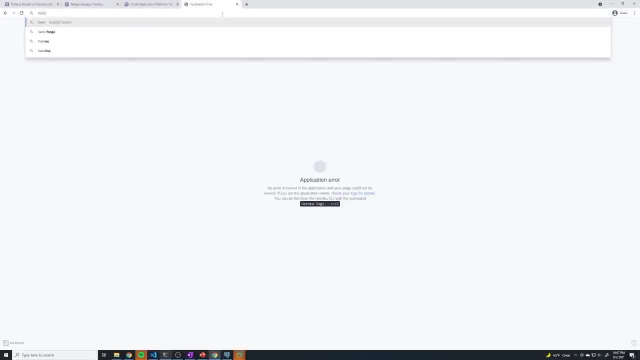 with a free Postgres instance that we can have access to, And that's what that's. one of my favorite parts about Heroku is that now we have access to Postgres, So let's go to Heroku Postgres. I'll just say tutorial. 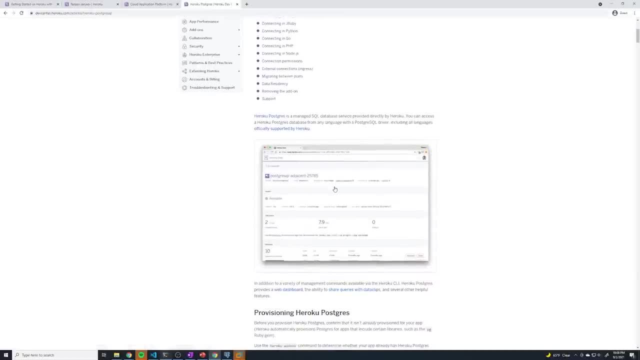 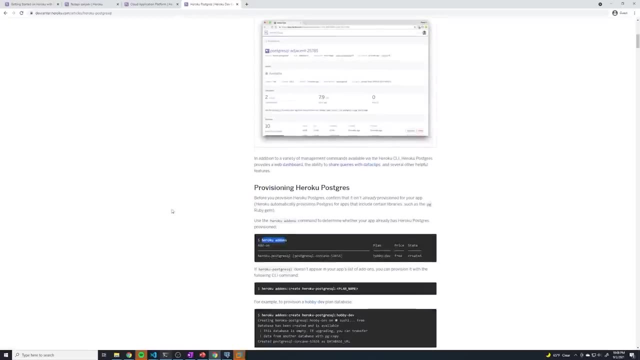 And it's gonna take us to their dev center. So this is going to show us actually how to create a Postgres instance, And so it. Postgres is one of their many add ons. if you want to actually go to their website and see all of the different add ons they support. 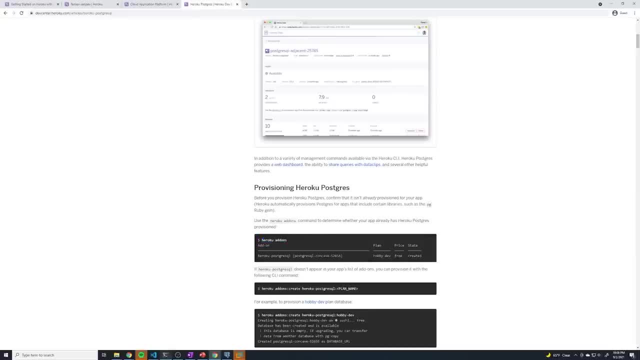 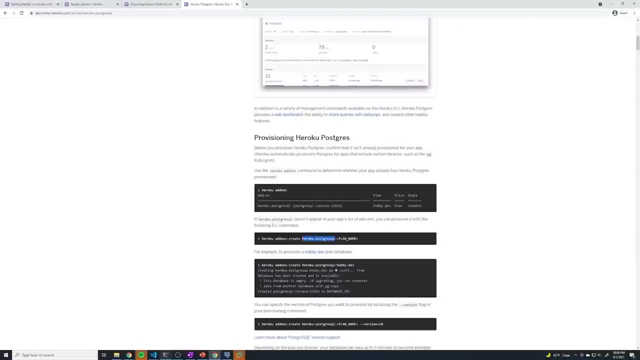 they support a ton. If you want to read this add on, you can get that added, But in this case we want to create a Postgres, a Postgres instance. So we do Heroku add ons. create then the type of add on. 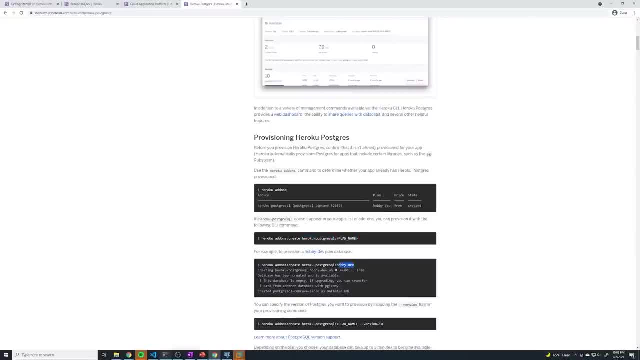 which means it's going to be Postgres QL and then plan name. So we are under the hobby dev, which is essentially the free one, And that's going to actually create a postgres instance. So let's run this and just Ctrl C out of this. 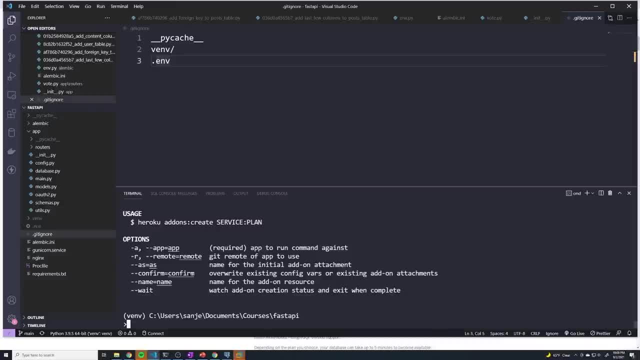 And let's just do a dash, dash, help real quick just to see what other flags we have, And that should be fine. We don't need to actually provide any other flags. Let's run this, And Heroku is actually going to create our Postgres instance, And keep in mind that for 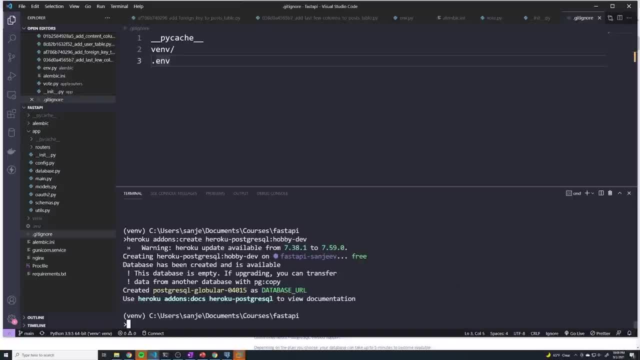 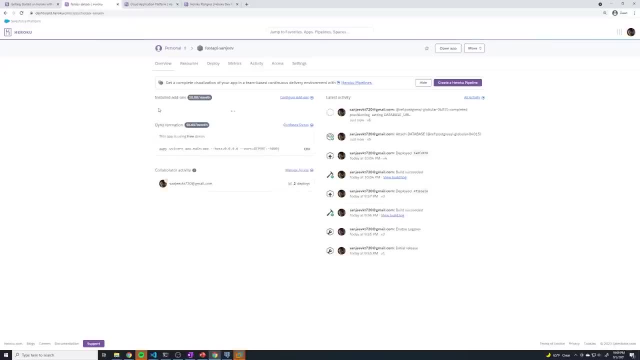 Heroku to spin up by Postgres instance. it does take a little bit of time But we can actually monitor that in our dashboard. So if we go back to my dashboard and do a refresh, you can see that this is the new Heroku instance. 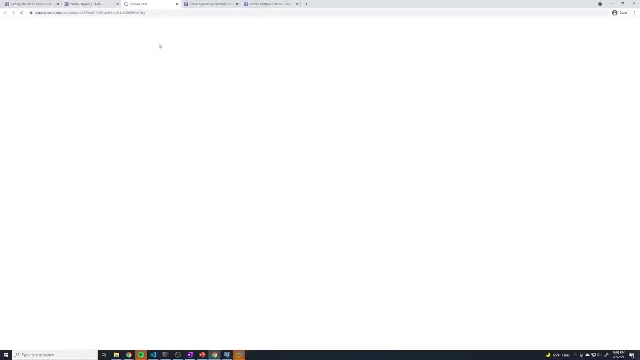 And I can just click on this and we can see some more information is going to open this up in a new tab And, if you want to, we can go into the settings And here we can take a look at our database credentials. So if I view my credentials you can see that this is the IP address my database lives on. 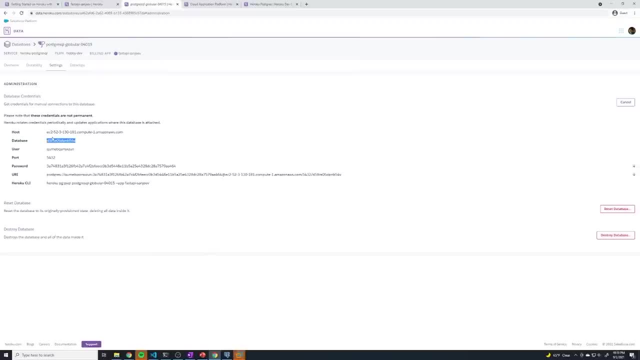 This is the actual database name, So we don't get to create our own database name or our own database within Postgres. they give us a fixed name, And that's perfectly fine. And then here's: this is going to be the username that we're going to log in, as this is the port. 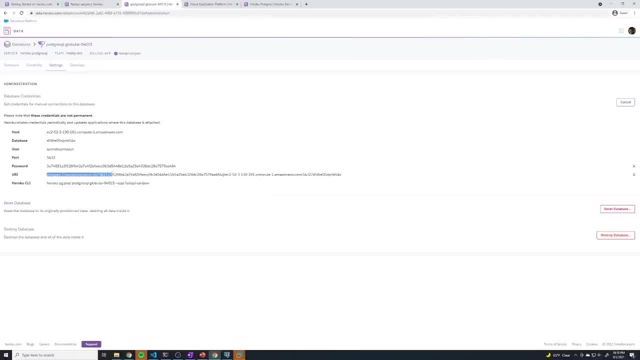 it's running on And then this is our password And they also provide us the full Postgres URL if we want to use that. So now that we have this information, feel free to save this real quick, And I'm actually just going to do a quick screenshot. 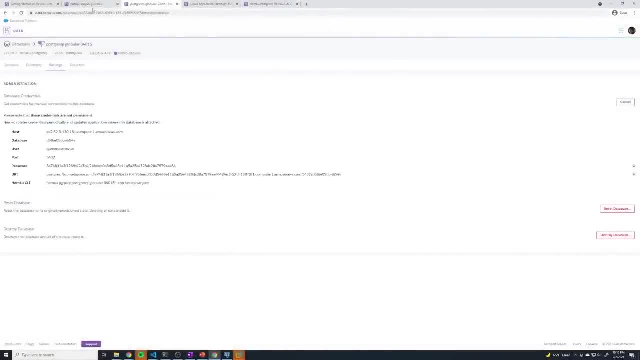 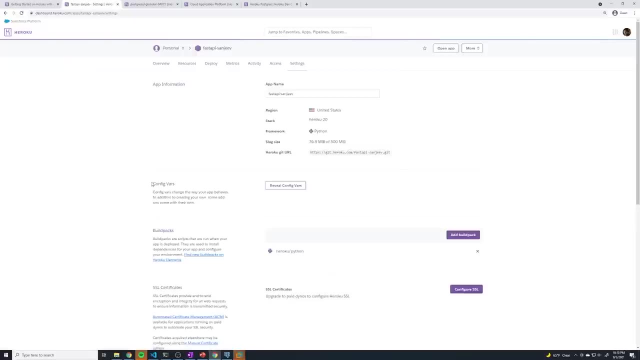 and save this in my notes so that I don't have to keep bouncing back and forth. And now let's go back to our application. And if we go under settings, this config vars is where we actually provide environment variables to our Heroku instance. 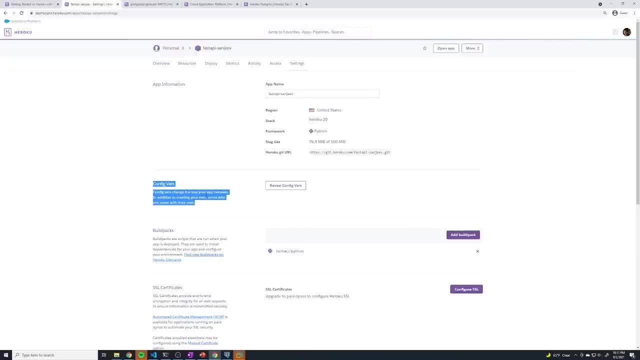 And, by the way, Heroku calls our instance dinos, But you can use either term you want, And so you can see all of the config variables that have been set, and there should be nothing except for one. So when you add a Postgres instance to your application, what happens is Heroku automatically. 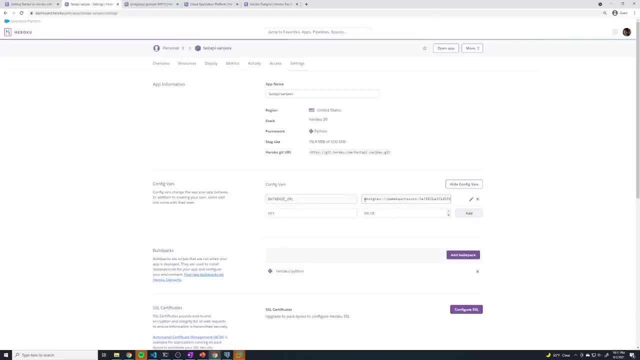 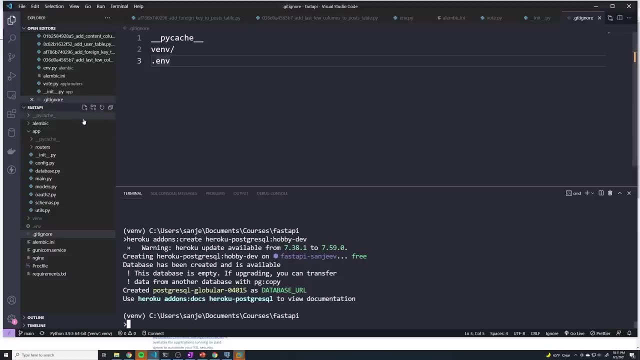 adds an environment variable called database URL, and it's going to contain the entire Postgres QL URL, URL, And so we could go into our application and then update our code so that in the database dot py file, instead of you know, breaking things down like this, we can just: 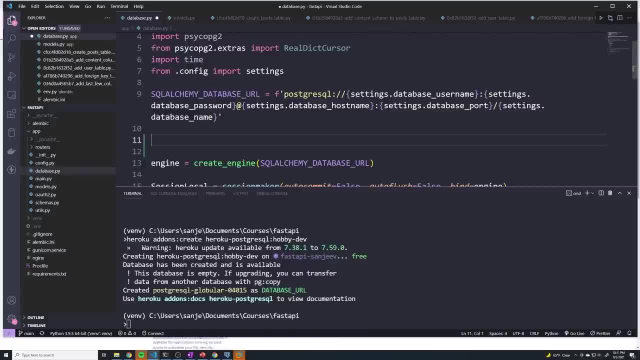 provide you know one, one specific URL and just put it in as settings dot. you know database underscore URL. However, I don't like to change my code. I like it just the way it is. So, instead of using the default environment variable, we're going to actually break this. 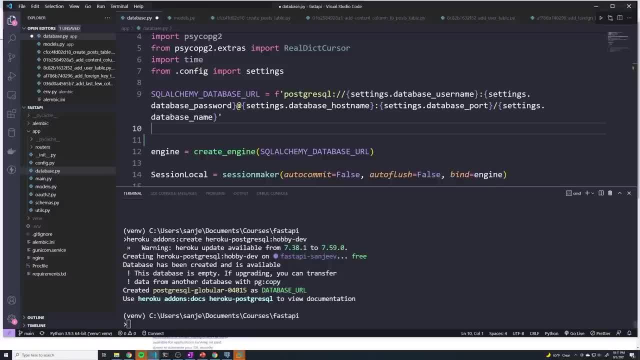 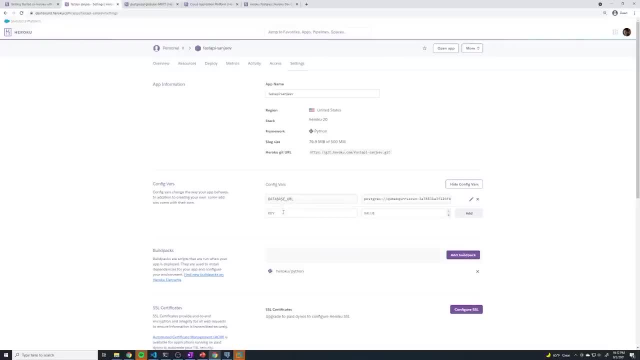 URL out into multiple different environment variables. So just open this up and take a look at all of the environment variables that we expect by going into our config dot py. So we need all of these set. So we're going to add one for database hostname. 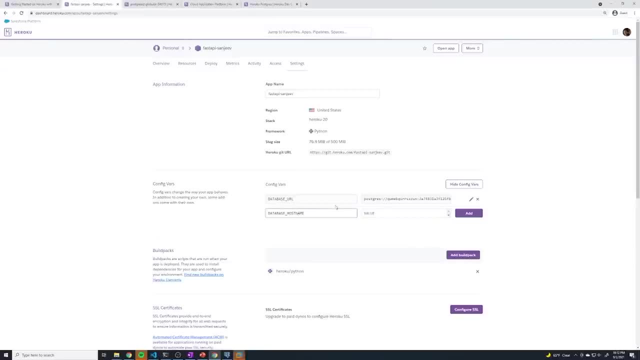 button button, box box, page box box inbox. forgot what the host name is And actually I'm going to just open this one up in a new tab And then open up. actually I don't even need to open up this one, I just need to flip. 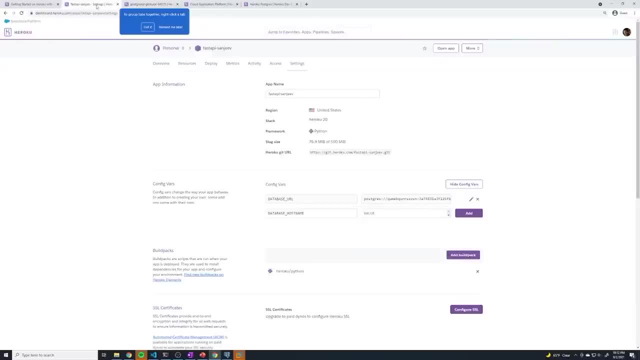 between these two. So the host name is right here, And but you can get it from this URL just by clicking on this icon and then just grabbing the IP address. But it's such a small little window I hate having to do that, So I'm going to close that and just bounce between. 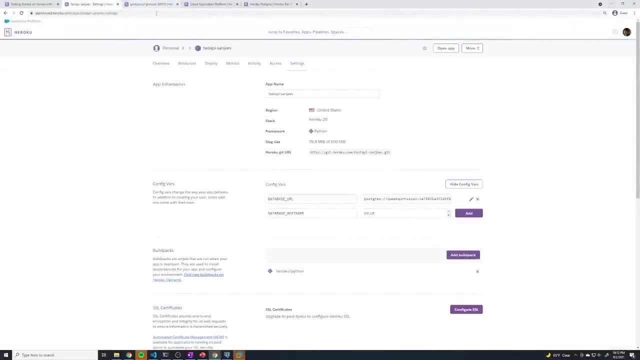 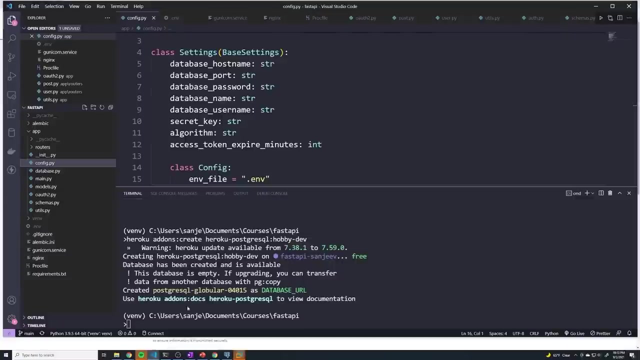 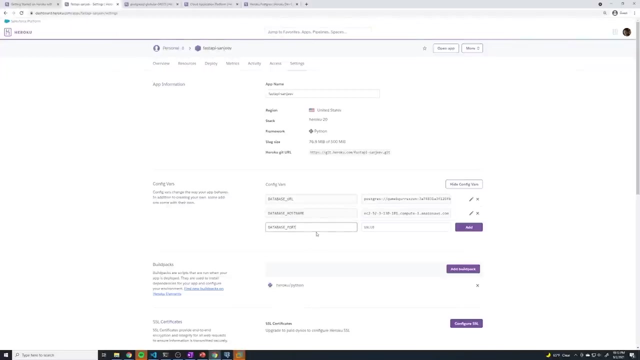 these two links. Alright, so let's grab the host name And we'll add this one. then the next one is going to be the database port password, name and username. So let's just write those out: database, Database username, Database password And then database name. I think that's it, Database. 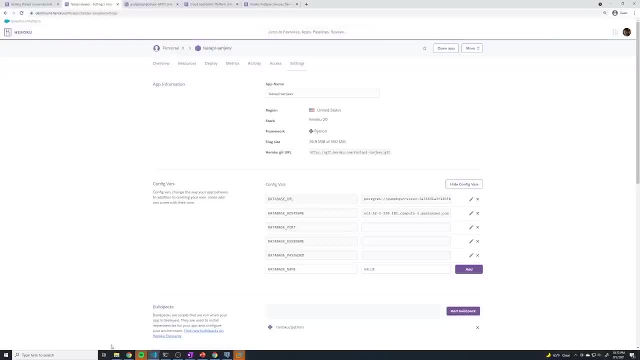 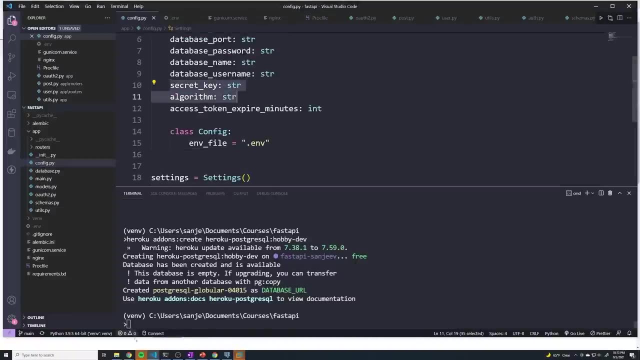 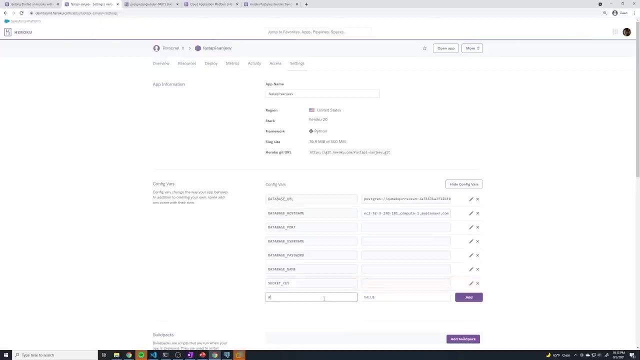 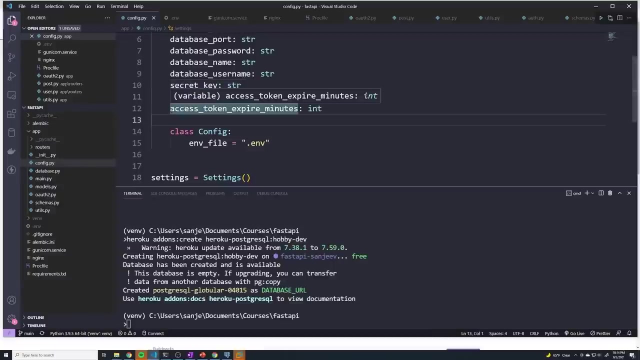 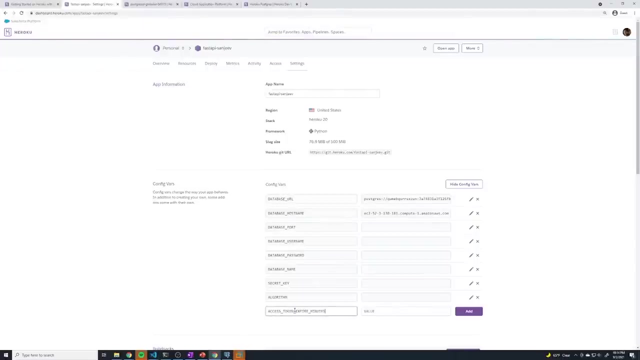 port, password, name, username, And then we have to add this stuff for our table, And then we have to add this stuff for our table, And then we have to add this stuff for our token. So we got secret key algorithm. and then the last one. 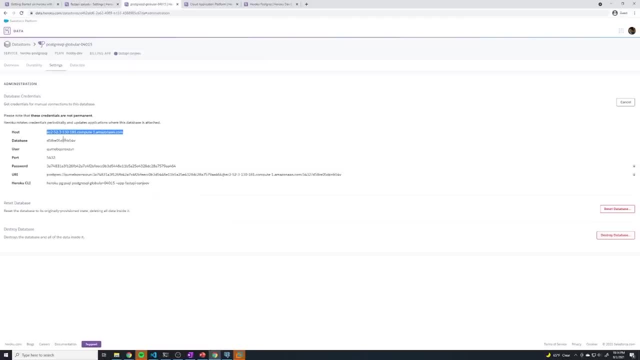 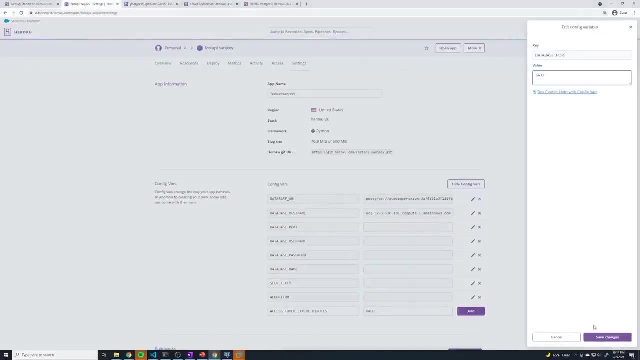 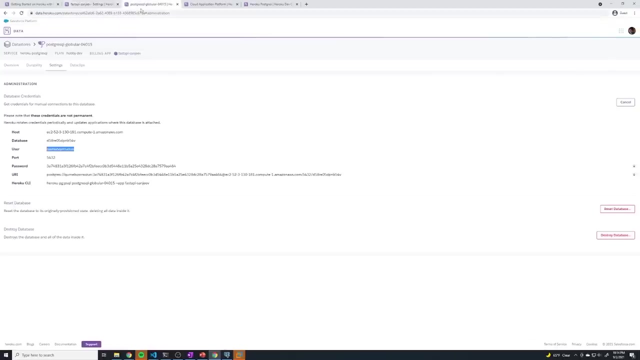 And then now we can provide in the value So the database port we can see from here. it's going to be the default About 5432.. The username, And then here we'll grab the password. And then here we'll grab the password. 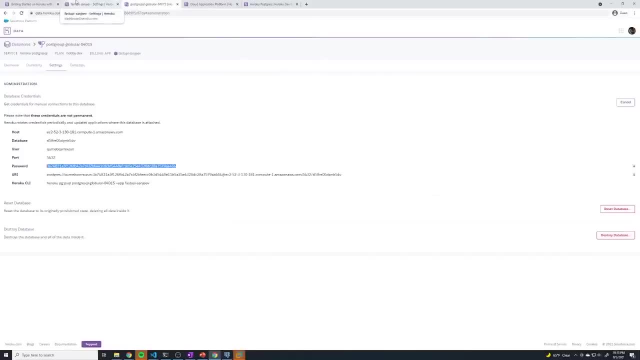 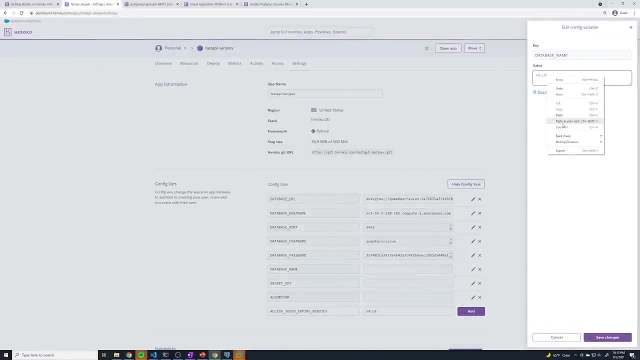 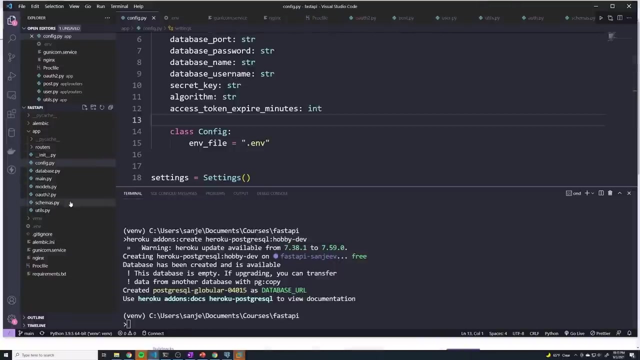 And then the actual database name here, The secret key. I'm just going to use whatever we used in development- not actually recommended, but I'm just going to keep things as simple as possible for now. But you can provide any secret key you want. 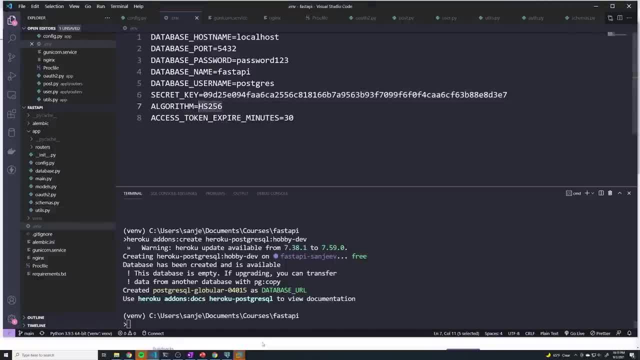 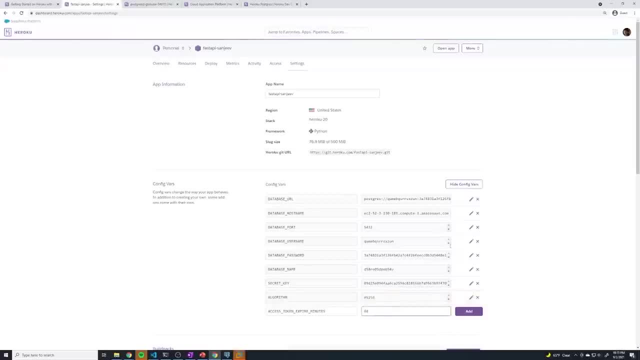 And I'll say in production, it'll expire after 60 minutes. Alright, and so now we've got our all of our environment variable setup and our Postgres Postgres instance is already up and running. So I think at this point our app should work. 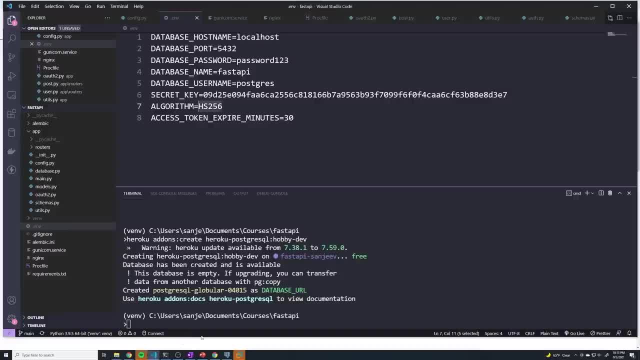 So we'll try this out again. So, now that we set those new environment variables, how do we actually restart our Heroku instance? Well, let's do a Heroku apps dash, dash help And let's see if there's a restart. 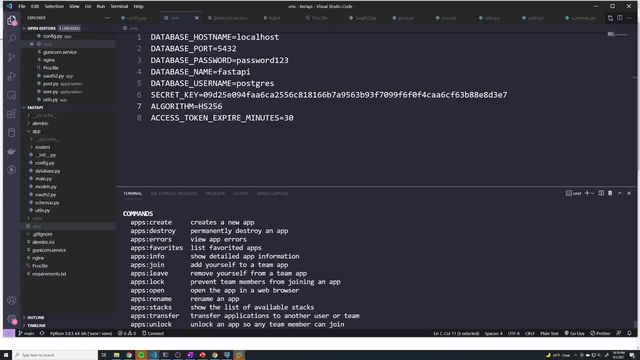 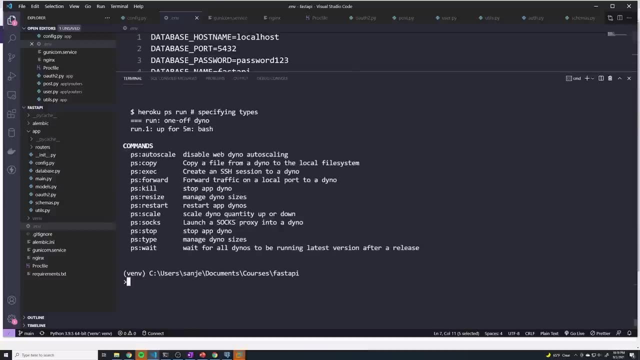 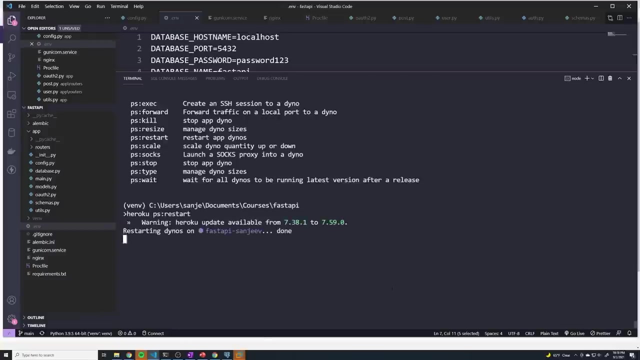 So there's app create, destroy. It doesn't look like there's a restart, So we can actually use the apps argument to restart our application. Instead, we have to do Heroku PS dash help. So now we can see that we do have access to restarts. we're going to do Heroku PS restart. 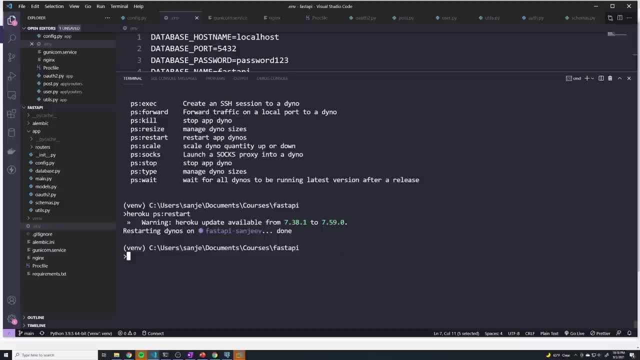 And that's going to restart our dyno, which is our Heroku instance, And once again I'm going to do a Heroku logs dash T to tail the logs. Alright, and so now you can see, those previous errors are gone. 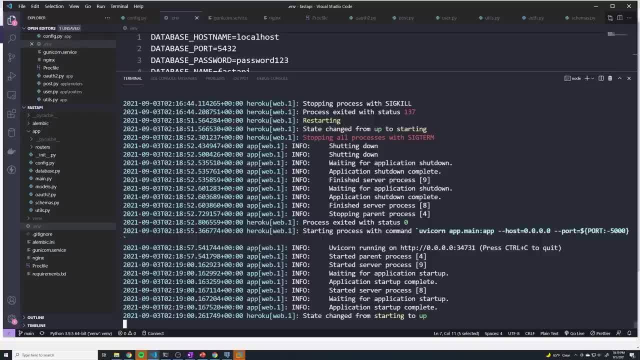 And we were now able to successfully restart. So let's go ahead and run the startup command And you can see that we actually got past a specific port of 34731.. And so that's why we ultimately had to provide the port variable, because this will change. 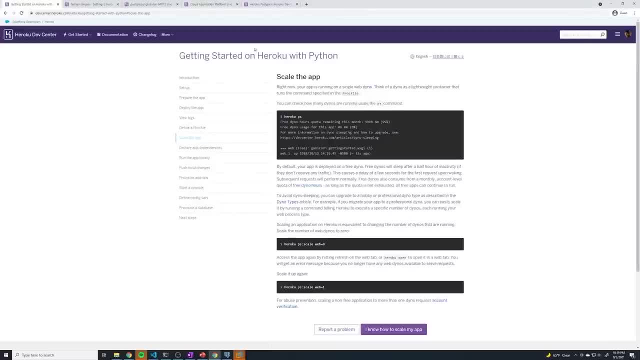 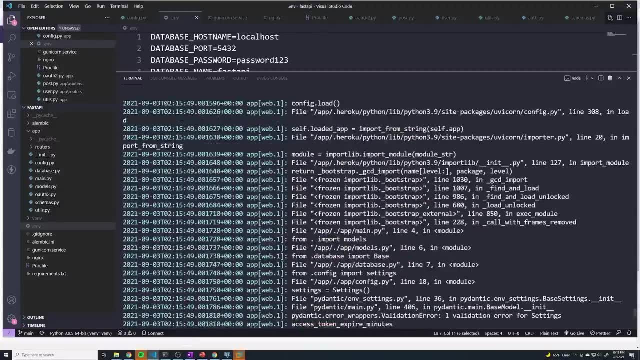 every time we restart it. However, we don't actually need to use that specific port number in the URL that we need to access, So let's get our our app URL, which I already forgot And if you've ever forgotten, I'm sorry. 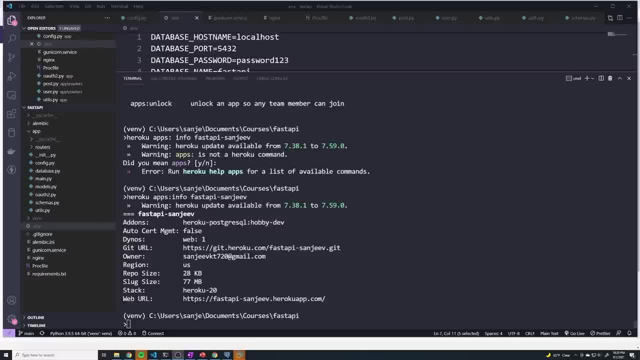 I'm sorry. I'm sorry, Don't forget your URL. you can just type in Heroku apps info than the name of this specific app, And then it's going to give you all of the specific information, So you can see. this is actually where the Heroku get is being stored. 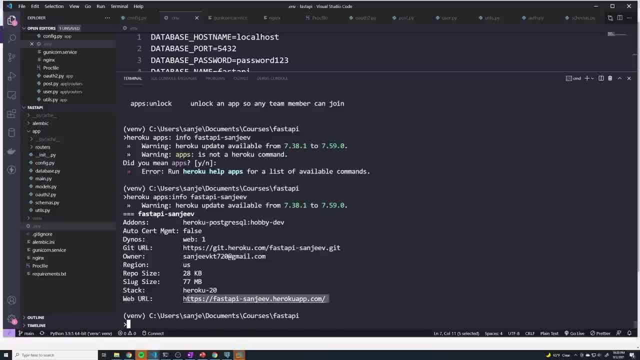 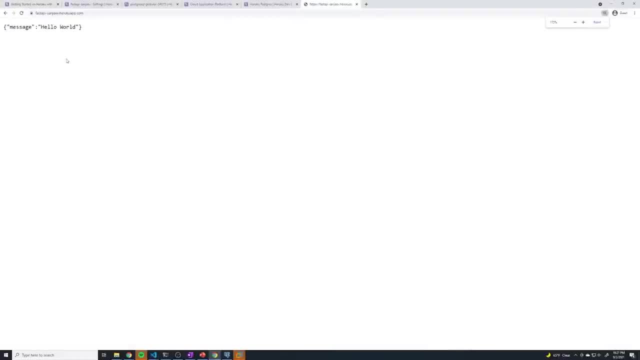 We can see that we have one instance in this case running the web And then we have our URL down here. So I'm going to copy this And you can see that we get message hello world. so it looks like things are working If I actually go to slash Docs. let's test that out. 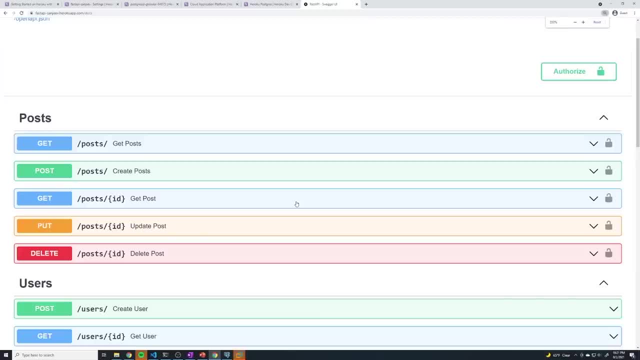 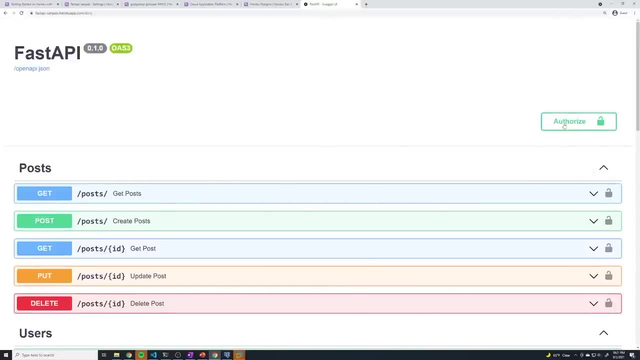 And so now we have access to documents. I'm going to minimize that So it looks like things are working. However, if I try to log in, whether it's either through the documentation or if I actually send a request from postman, you're going to see that there's going to be some issues. So 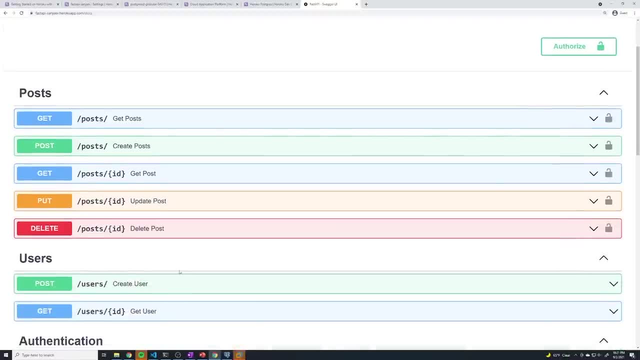 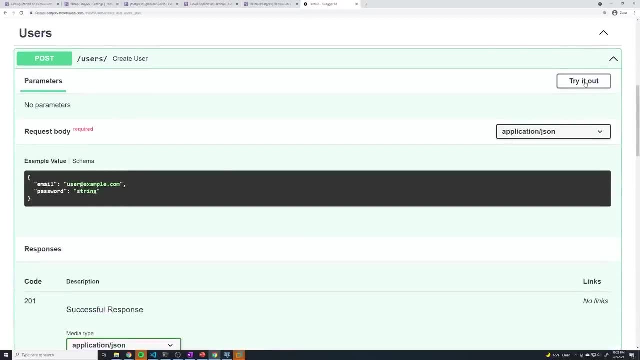 here I'm going to. actually, I can't even log in. I have to create a user first, because this is a fresh deployment. So let's go to users And we're going to create a user real quick And I'm going. 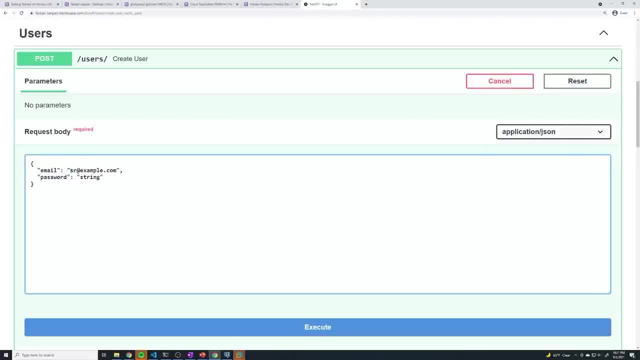 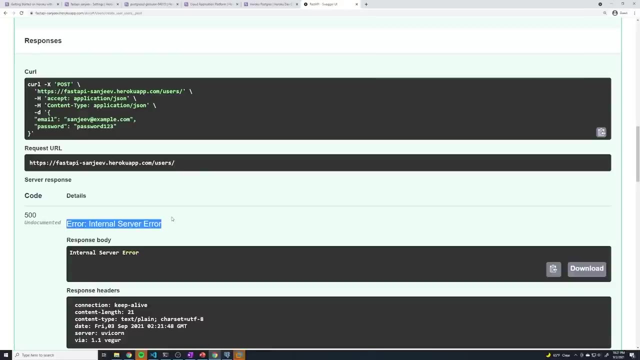 to just try this out and put in whatever name you want Now. so this is Sanjeev at examplecom. my password will be password 123, we'll execute it And you can see that we get an internal server error. So what is happening? Why can't we exactly create a user? Well, like usual, we're going to go. 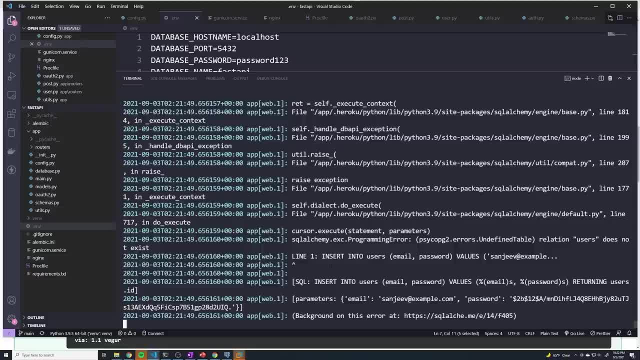 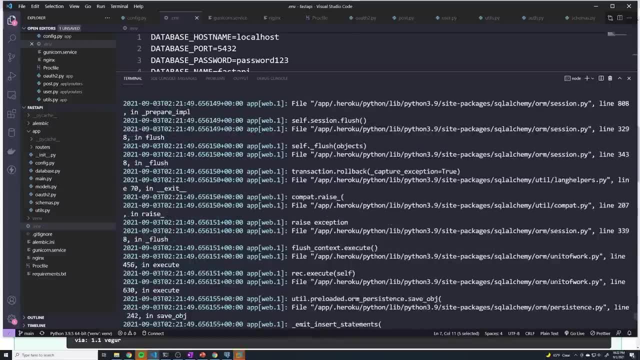 back to our logs And we're going to see what happened. Alright, so we can see the SQL that's getting inputted In the logs And it looks like there's some kind of error with the SQL, And I don't know if that's. 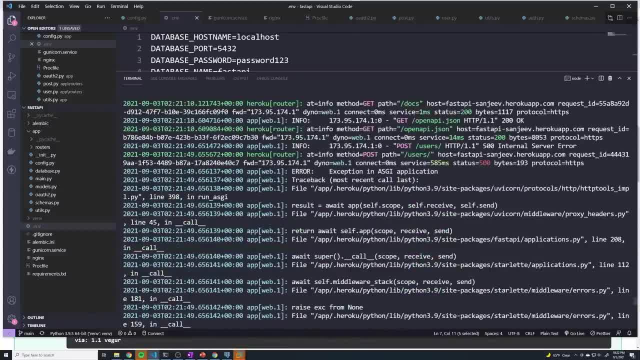 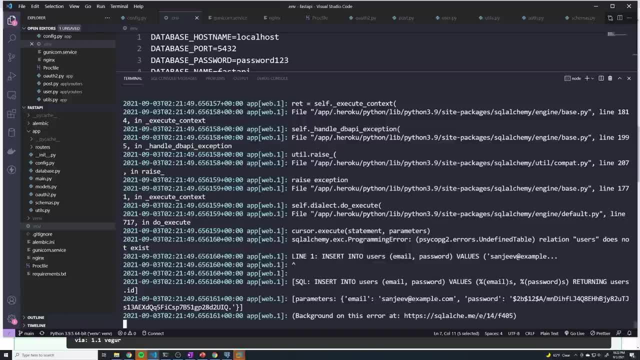 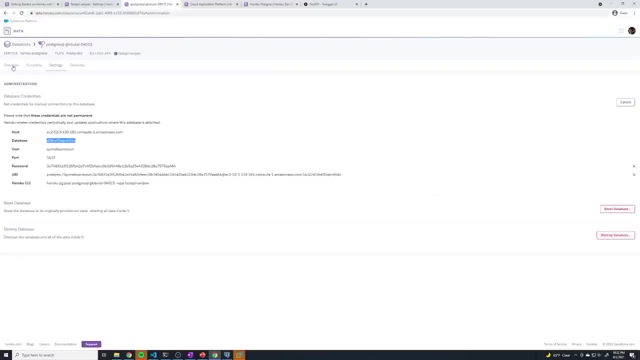 going to give us a more specific area that's going to actually help us. I think that's all it's going to provide us in this case. But I think you guys can guess exactly what's happening. We deployed a brand new instance of Postgres, But right now, if we actually connect to our Postgres, you're going 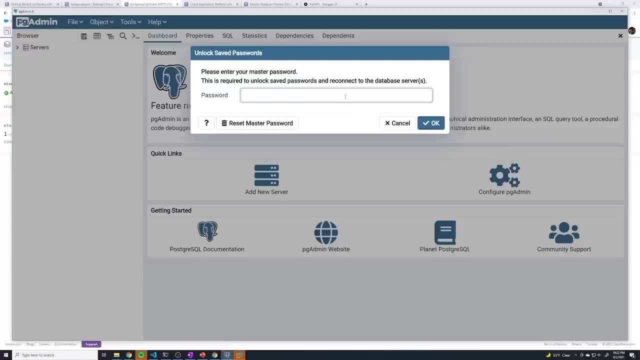 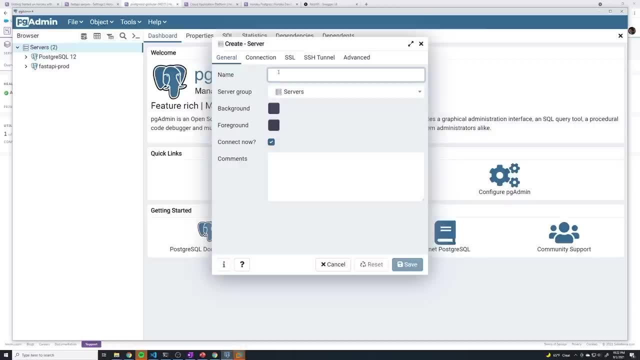 to see a few different issues. So I'm going to actually connect to this Postgres instance And to create a Postgres instance, just right click here and then select Create server. So this is going to allow us to connect to another Postgres And I'm going to call this Heroku dash Postgres And then here. 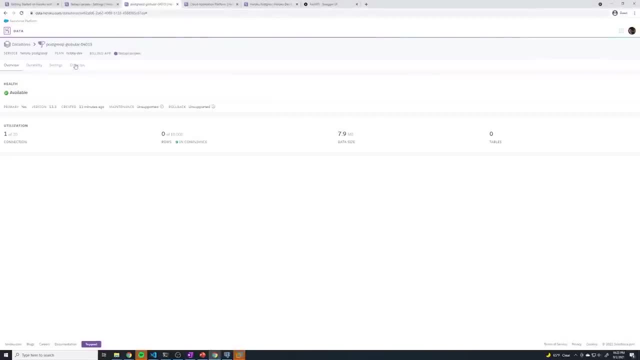 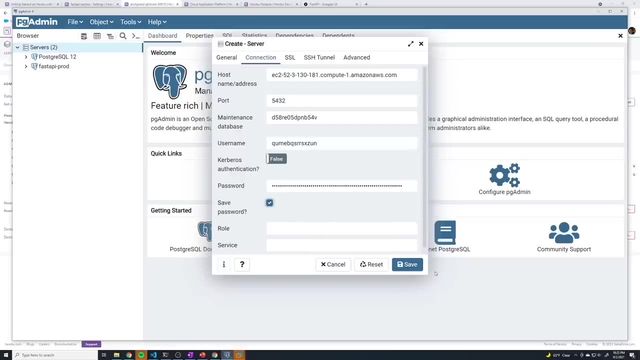 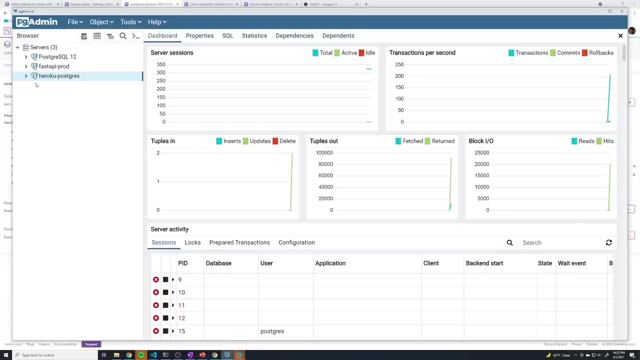 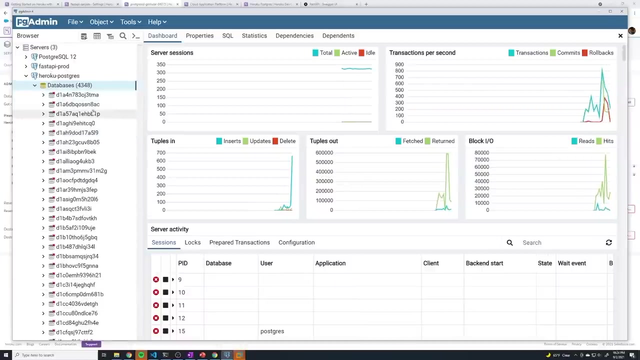 we're going to provide the same exact connection information. We'll go back to settings. we'll get our credentials, Okay and so now we are successfully connected to to our Heroku Postgres instance, And if I just drop this down and then go into databases, you'll see a ton of different databases. Keep in mind, we won't actually 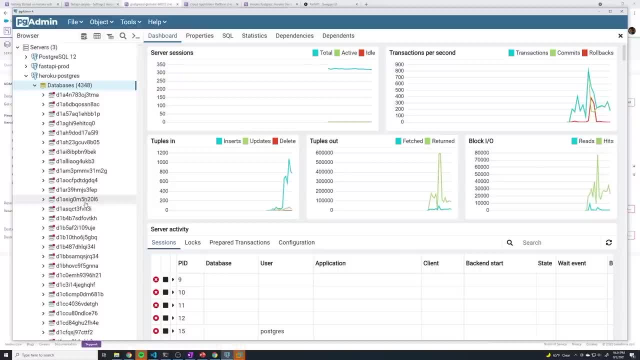 be able to access most of these. So the reason Postgres is able to- sorry, the reason Heroku is actually able to provide this for free, is that they have one instance of Postgres And then they give you one database within that instance that you can access, but only you can access that. 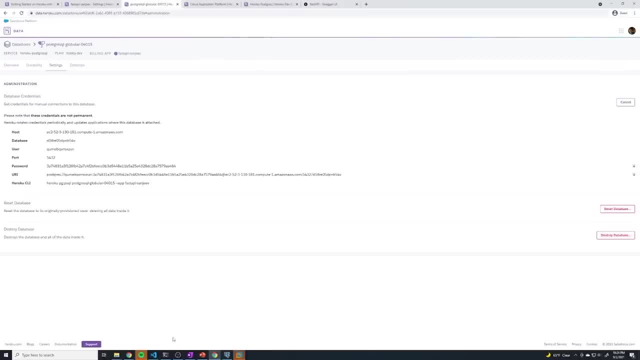 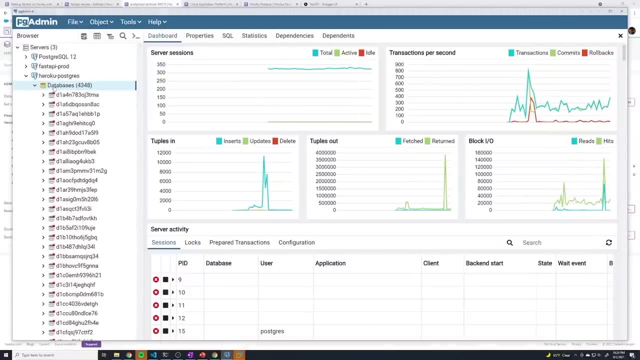 specific database, And so our database is d58.. And I don't know if there's an easy way to search for databases. Let me see if I can right click this. Nope, it doesn't look like there's an easy way. So 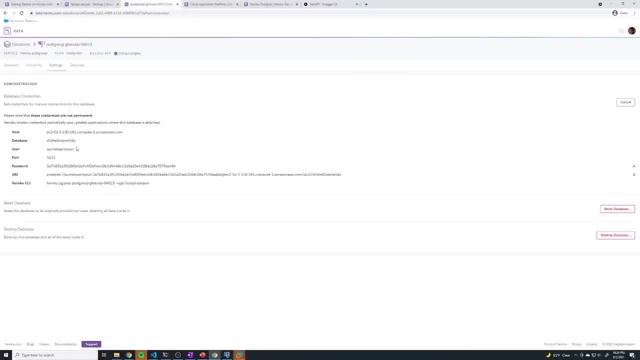 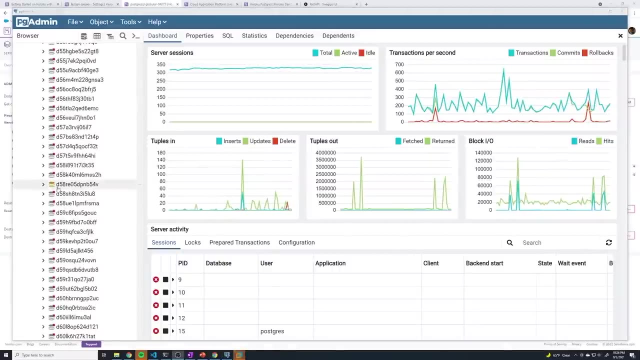 I'm just gonna have to scroll down to d5.. And then what are the next letters? d58, re05.. Alright, so I finally found my database. you'll see, it's the one that I have access to, So it's actually colored. 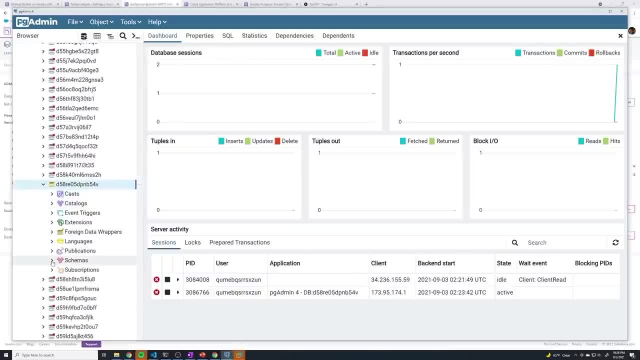 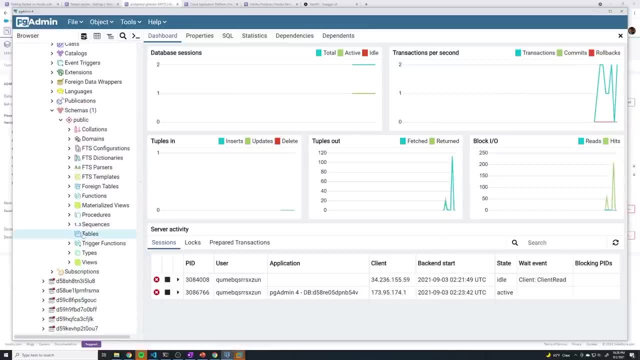 And if I just open this up real quick and go into schemas- public- and then tables, There's nothing in there. So that's really the reason why our application is not working is because we have a brand new Postgres instance, But we haven't actually set up our tables or our schema, And so this is where Alembic 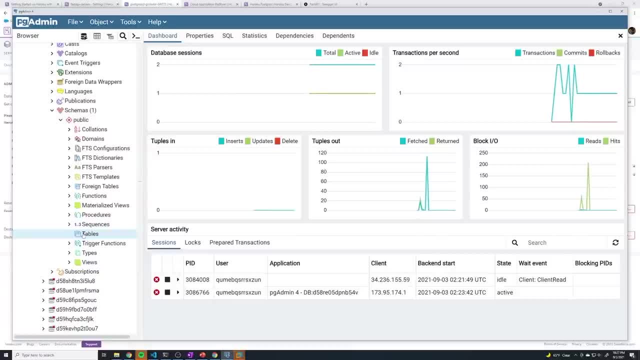 is going to come into play Once again. you'll see that, since we already have all of our revision setup, getting our production database to match our development database will be as simple as just running one simple command. So we'll take a look at that in the next video In our development. 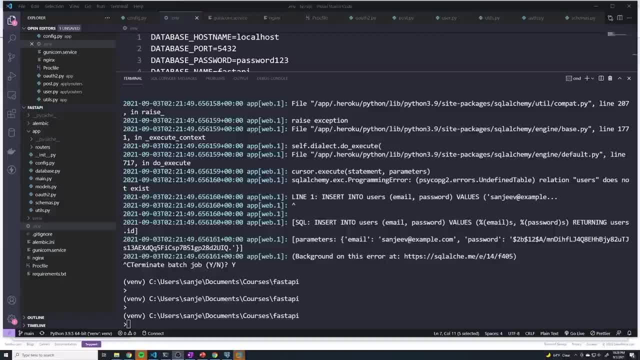 environment. we used Alembic to manage our database schema, So Alembic was responsible for creating all of those tables And since we have all of these revision files within the Alembic folder, we can essentially track all the changes that we make. 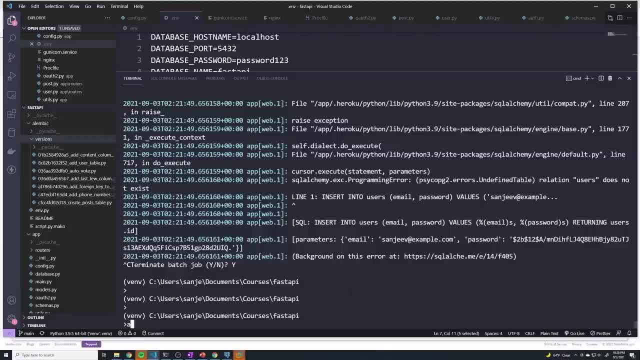 And so to actually get our development database up to date, we just ran Alembic upgrade head and that would go to whichever one of these is the latest revision and make sure that our Postgres instance matched whatever that is in our production database. 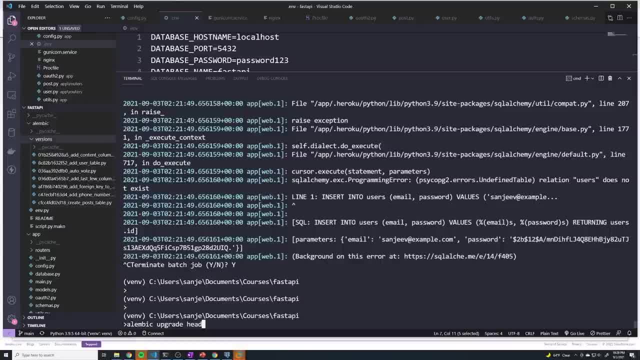 Because in our production database it's going to be no different. we're going to just run Alembic upgrade head on our Heroku instance And that's going to ensure that our Postgres database gets updated to our latest schema, And because we've checked all of these files into git. 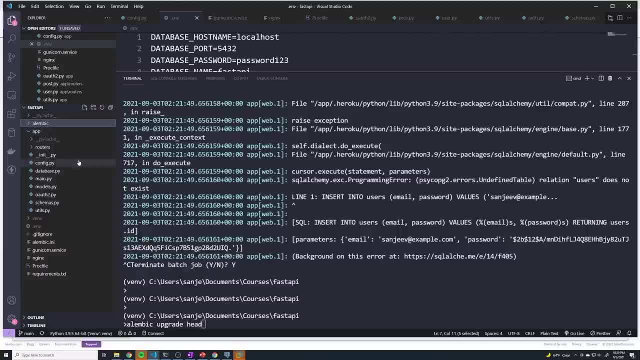 because all of the Olympic folders was added to get as well. Speaker 2. Then our Heroku instance has access to all of our revisions, And so when we run Alembic, Alembic can keep track of all of those changes as well in our production server. 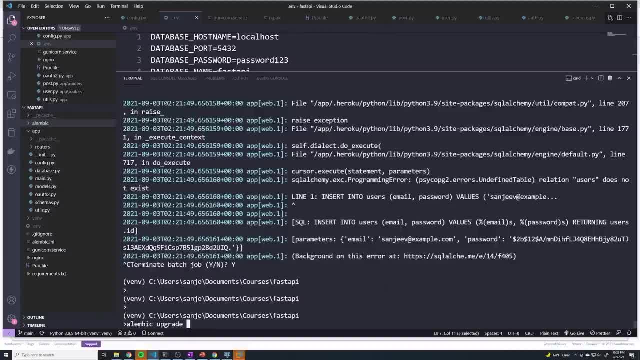 And it's important to understand that we never run Alembic revision on our production server. We only run Alembic revision on our development server when we're staging out these changes In our production server whenever we want to push out those changes. 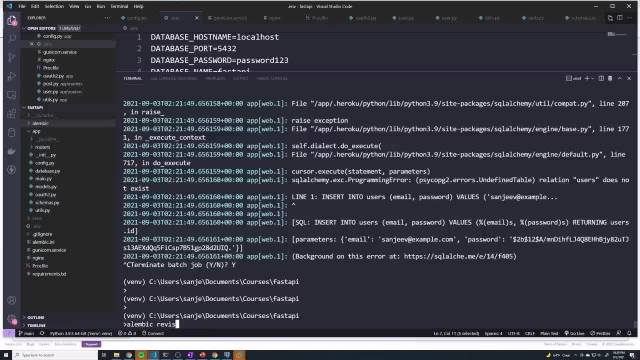 we just do a git push, So we push out the code, all of our code changes, as well as all of the Alembic revisions to our production server and we just run an Alembic upgrade head. It's as simple as that. So let's do that now. The first thing that we need to do is we got to figure out how. 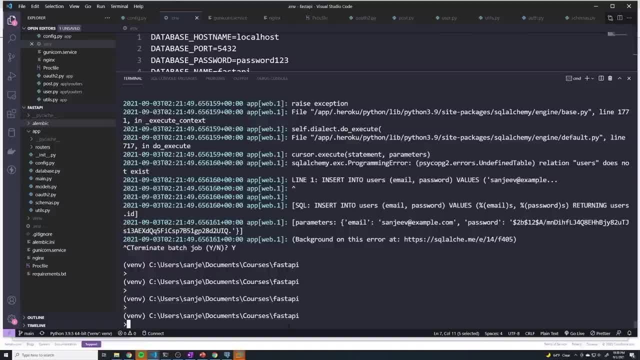 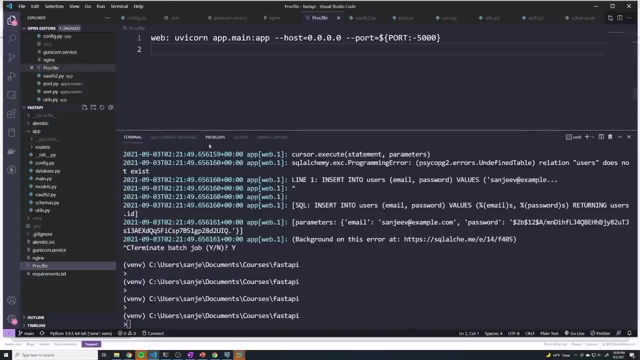 do we actually run a command in our Heroku instance? I think your first guess is probably going to be: do we add another line into this proc file that we can kind of call whenever we want to? Not exactly, although maybe you can do that, But if we go back to our tutorial and go to start a 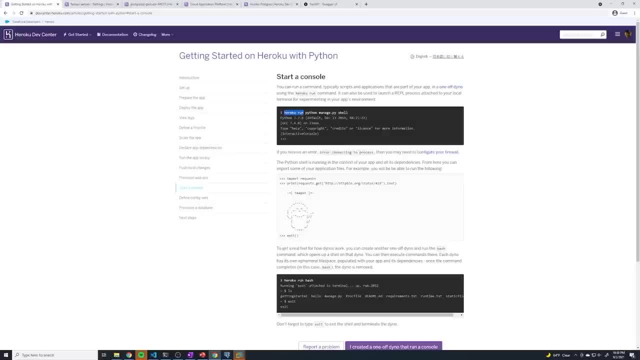 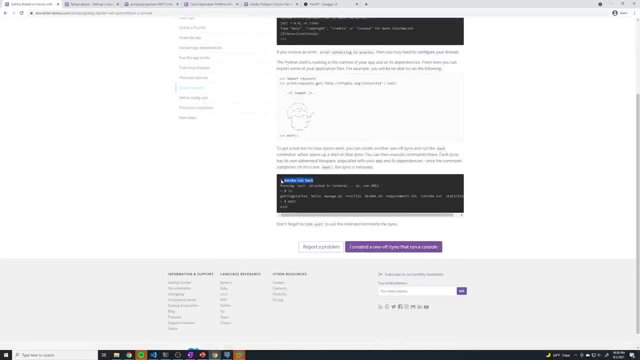 console. we can run a specific command on our Heroku instance by doing Heroku run and then the specific command that we want to run. So let's try that out. And you can even drop into the bash shell. So there's a lot of flexibility. 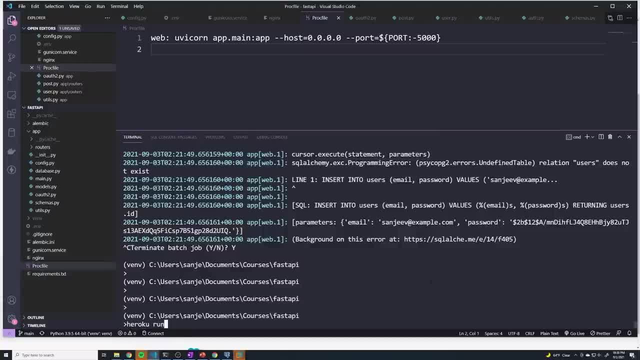 But we're going to just do a Heroku run And then we want to provide the command that we want to run. I'm going to put it in quotes. I don't remember if it's a requirement to put it in quotes, But I'm going to do that just in case we'll do Alembic upgrade head. 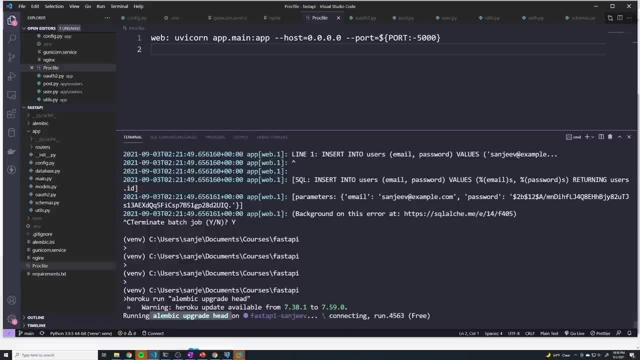 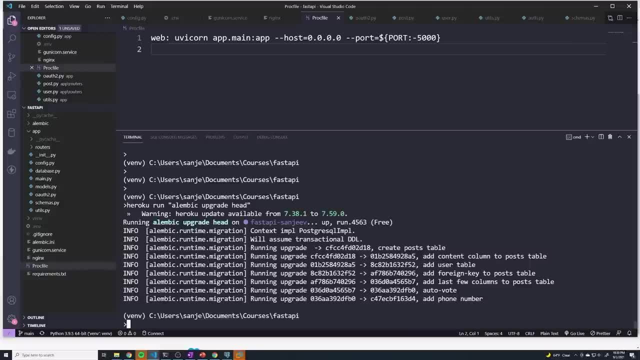 All right, and you see that it's running that command right now. And take a look at the logs right, you can see that not only did it get our Postgres instance up to the latest revision, it has all of the other incremental steps added in as well, So we can roll back to any of them. 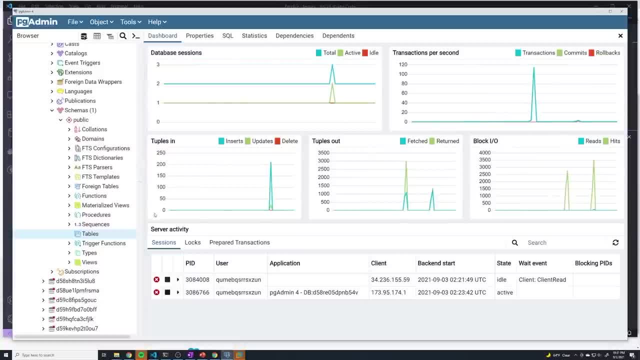 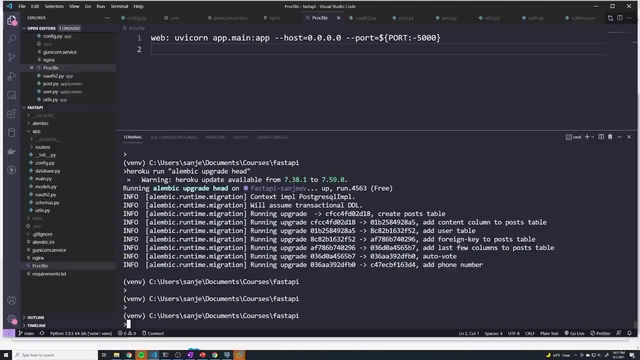 just like we did in development. And if we go back to PG admin, I'm going to just refresh tables And if we go to our tables, you can see that we have all of our tables here now. And just in case, because I believe we crashed our application, maybe when we try to, you know, 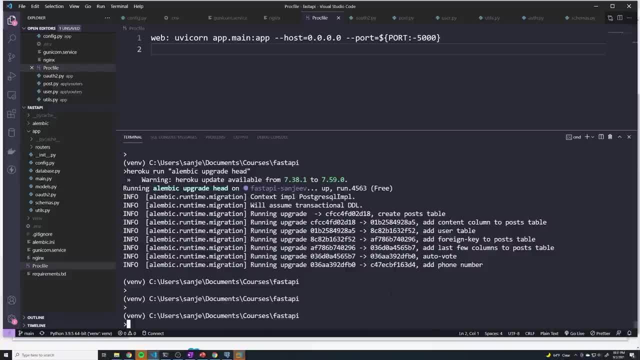 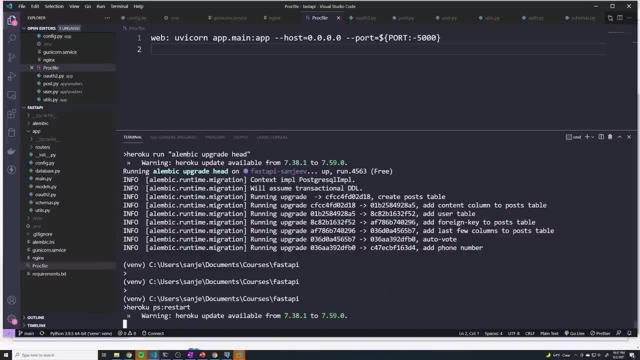 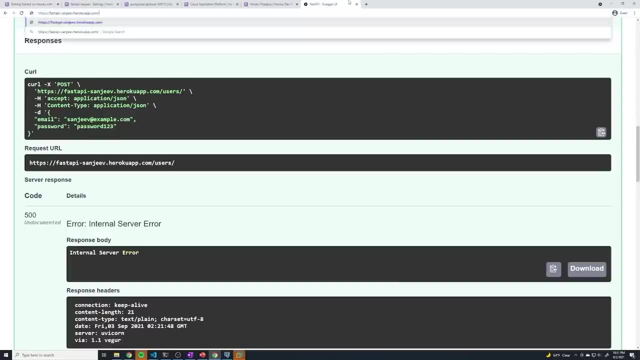 create a user without having a Postgres database or table setup. I'm just going to do a Heroku PS restart again just to restart the instance, just in case. And now I want to go back to here And we're going to just go back to the root URL to see if that works. And that works, That's perfect. 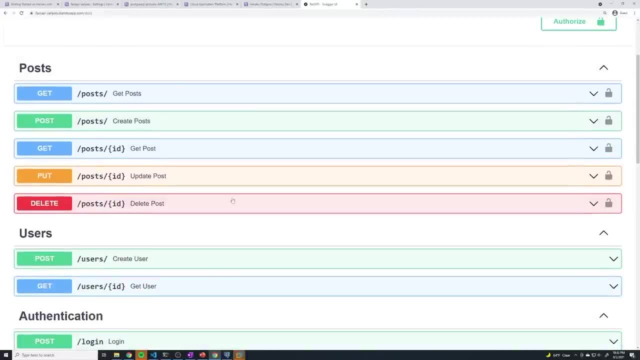 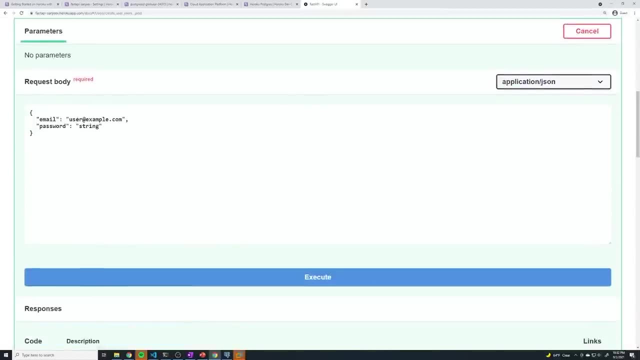 We'll go back to docs. We can see that that works. Now let's try to create a user, And so I'll do try it out, And I don't even feel like changing any of these values. Technically, these should still work. 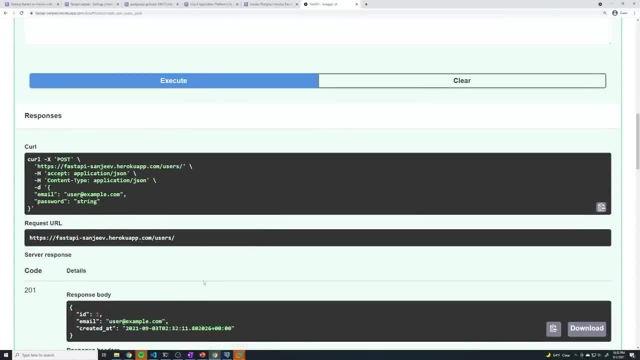 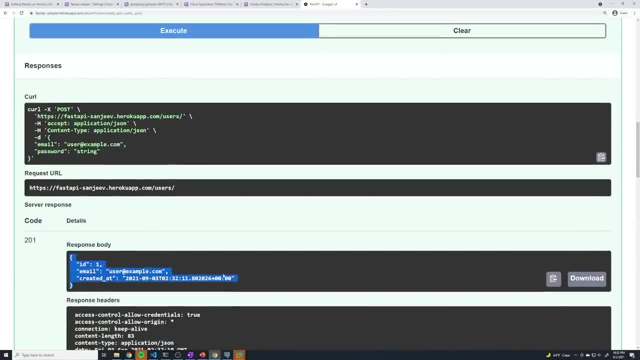 So let's just try that. And we got a response back. And look at this, we got a 201.. And we can see the user that was created. So it looks like our application was now successfully able to access our database. If we go into the users table, right click on this and just do a view: edit all rows. 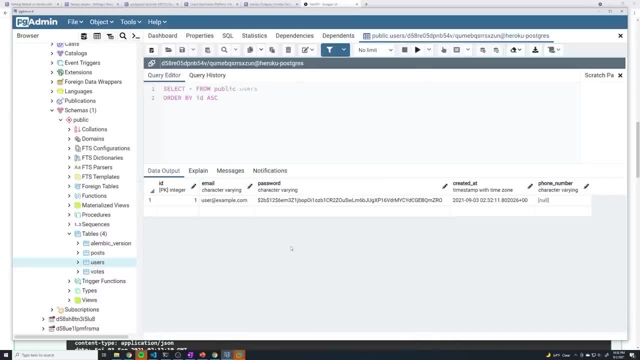 We can see the one user that we created. Alright, and so that's pretty much it. we've successfully deployed our application. The last thing that I want to show you guys is how do we push out changes to our application. So let's say that I go into my app And right now I go into. 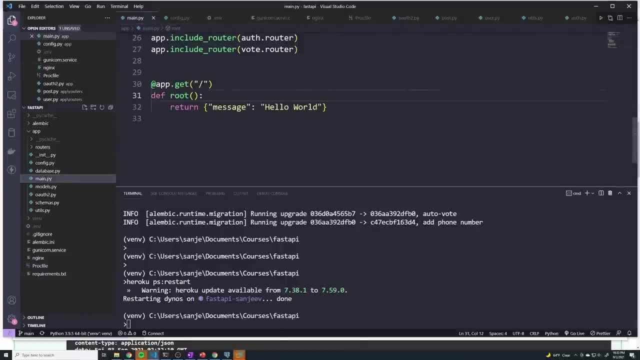 mainpy, And I see that this just says message, Hello world. And let's say I make some kind of change And let's say I just add a whole bunch of exclamation points or something, just keep it. keep it simple, just to show you guys, you know, regardless of what change you make, 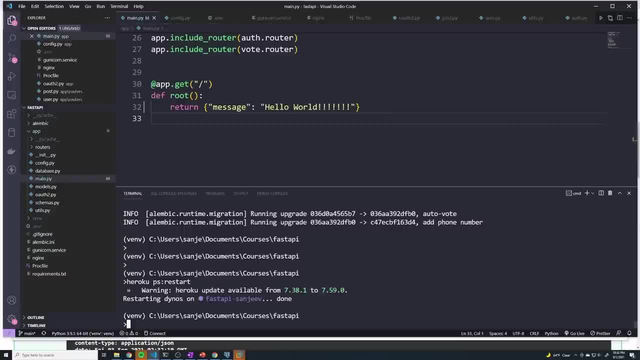 the steps are going to be identical: we make some changes And the next thing that we have to do is we actually have to push out those changes. So, first of all, you're definitely going to, you know, push out those changes to your GitHub repository, So we'll do get. 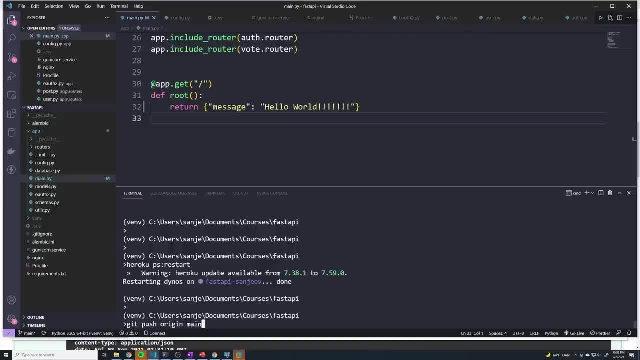 push origin main. So that's going to push it out to get GitHub. Well, sorry, I forgot to do a git add dash, dash. also, we actually have to add those changes and then commit those changes. So we'll do git commit. 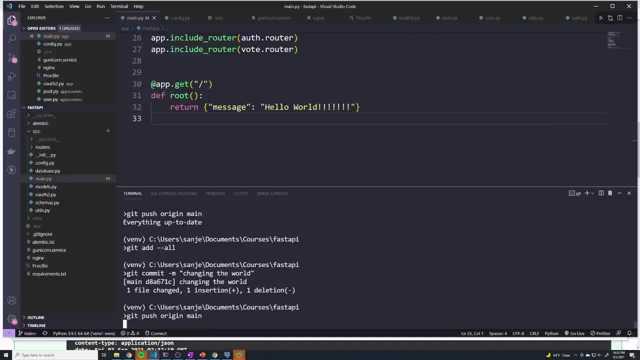 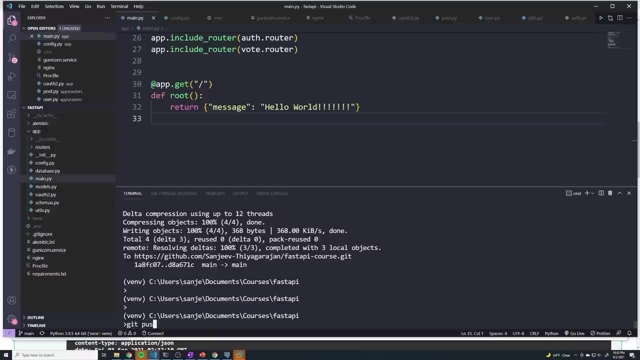 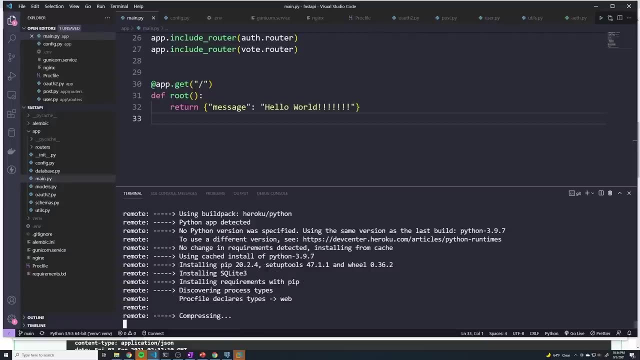 Then we'll do a git push origin main that's going to push it out to GitHub And then, finally, to actually push those changes out toward production environment, we'll do a git push Heroku main, Alright, and so that's pushed out now. And if we go back to our application, 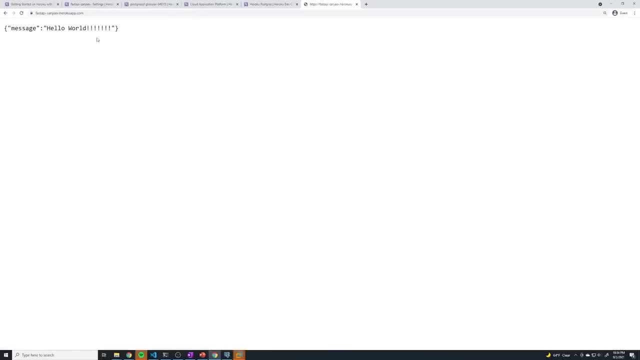 I'm going to go back to the root URL And we can see that we now have the extra exclamation points. So we have successfully pushed out our changes. all it took was just one simple command, And keep in mind that if you make changes to your code, that's all you have to do. 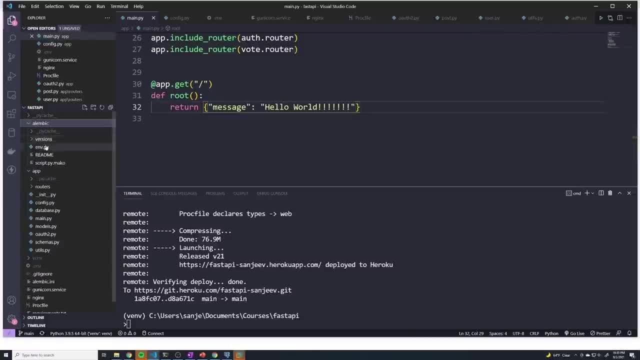 However, if you make changes to your database, so you know you go into Olympic and you create a new revision, then we have to follow the same exact steps, But on top of that we have to do the, the Heroku run, Alembic, you know, upgrade head, so that we actually push out those changes to. 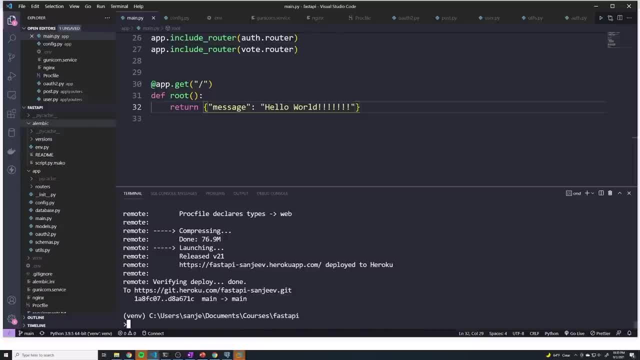 the Postgres instance. But there you guys have it. you have successfully deployed the application that we have spent building the past couple of days, And so feel free to show this off to your friends and family. Feel free to make as many changes, and modifications really start to play. 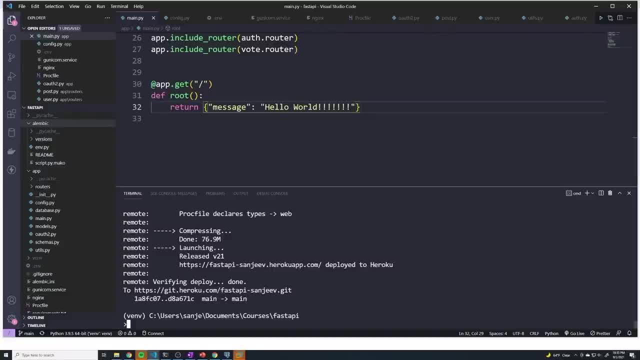 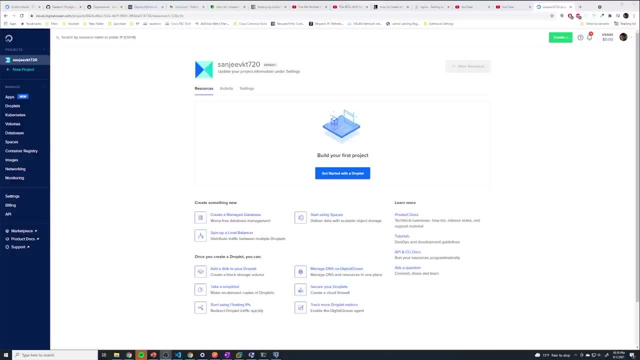 around with it, Try to expand on the functionality of our application And just keep learning. I guess for the second method of deployment, we're going to see how we can deploy your application on an Ubuntu server, And it's important to keep in mind that it does not matter where you host your Ubuntu server. 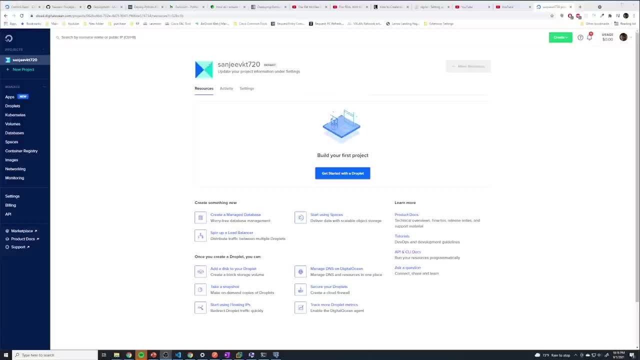 you can run it on any of the major cloud providers: AWS, Azure, GCP. you can run it on DigitalOcean. you can run it on your local machine. yeah, if you have VirtualBox installed on your computer, you can run it on Raspberry Pi. it does. 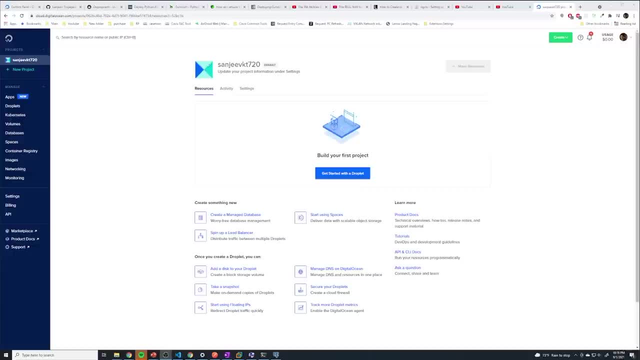 it doesn't matter, The steps are going to be identical, as long as you run it on an Ubuntu server. Now what we're going to do in this course is I'm going to show you guys how to deploy it on DigitalOcean. Just because it's $5 a month, it's cheap, it's a fixed price If you deploy it on AWS. 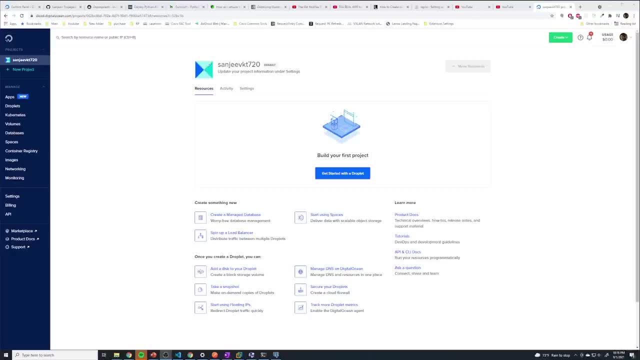 then the price is kind of it varies And if you run it all all month long then it could spike up well past $5. So this is kind of the cheapest solution. But keep in mind, like I said, the steps are identical regardless of where you deploy. 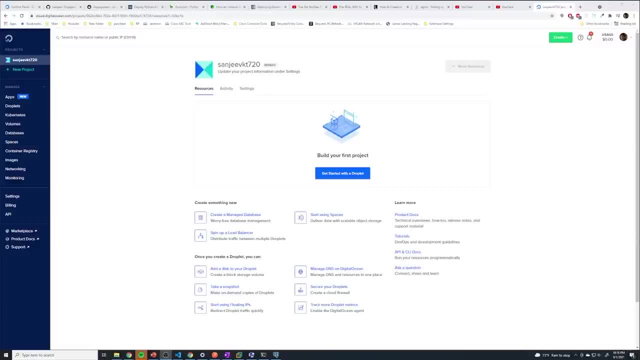 I just want to focus on making sure that you guys understand the steps that needs to take place to actually set up your Ubuntu server to be ready to host your application. And so, if you don't have a DigitalOcean account, go ahead and make one And then, once you log in, 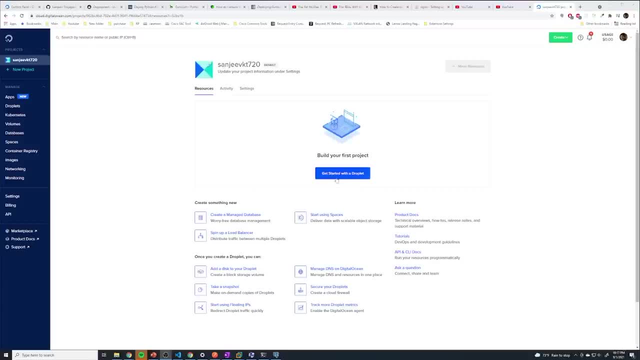 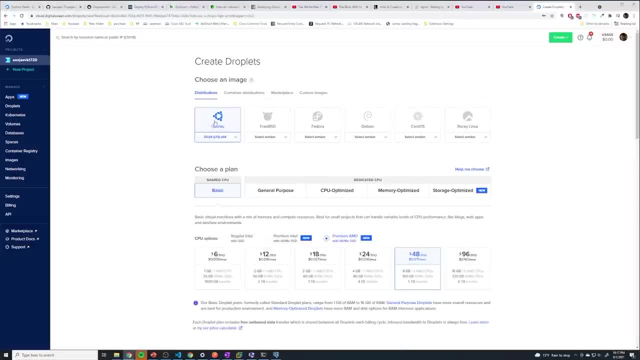 you'll see this window And what we want to do is select- get started with the droplet, So we'll select that, And what we want to do is we want to select Ubuntu 20.0.4.. That's the latest version at the moment. If you're watching this in the future, 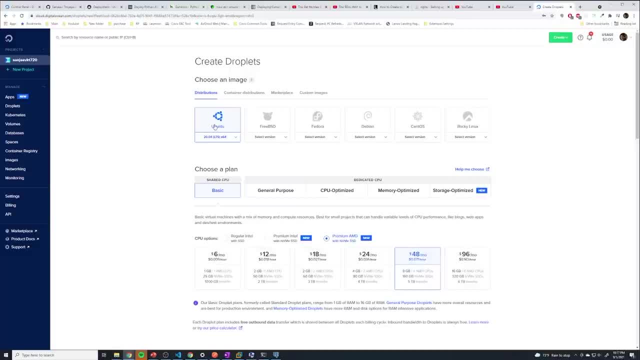 you could probably grab one of the newer ones. most of these commands are going to be identical, But if you wanted to make sure that you don't run into any issues, select the same exact version. Then, for the CPU options, you want to select regular Intel with SSD. 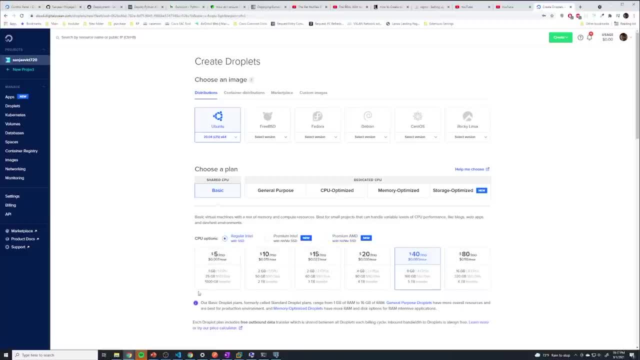 that's going to be the cheapest. And then you want to select the cheapest one right here, which is $5 a month or point 0.007 per hour. what is that? seven, seven tenths of a cent, All right. and then select your data center. So I'm just going to select whatever you want to do. 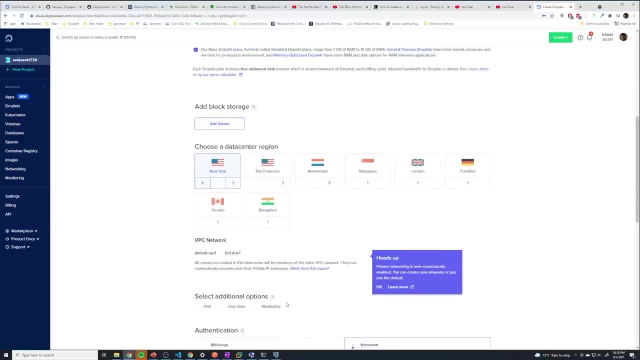 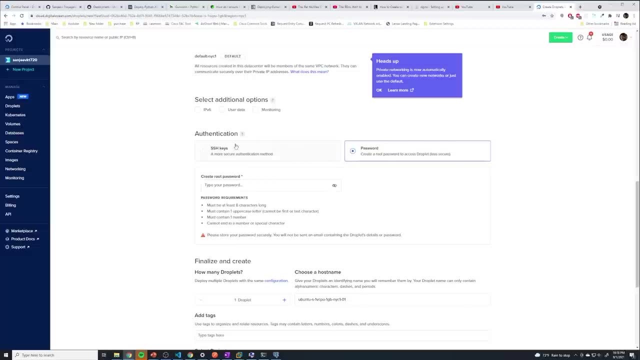 is closest to me- I'm on the East Coast, So I'm going to select that- And then nothing else, for the most part, really matters. we can leave everything as default, And then you have two options for authentication. you can use SSH keys if you're familiar with how. 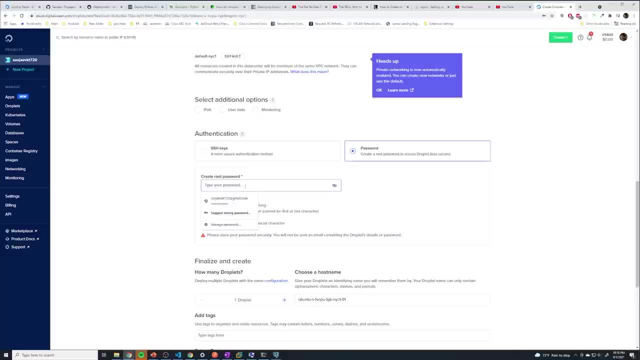 to work with that. If you're not, then start out with password, for now. it's just a little bit simpler, And you'll see that DigitalOcean has some strict requirements for passwords, So you're probably going to have to try this a couple of times before you find one that 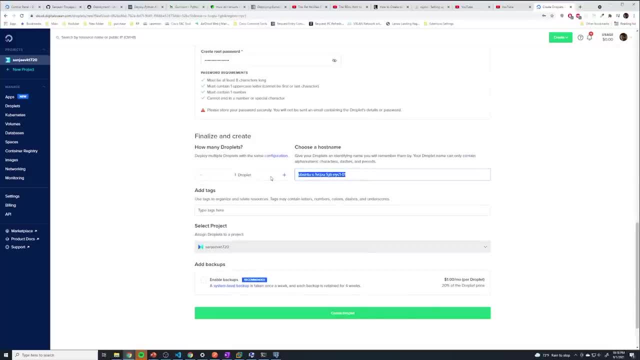 actually matches their criteria, And then here we can just give this a specific host name. I'm just going to call this Ubuntu dash fast API. It's nothing more than really just a tag, And that's all we have to do is select, create Doppler droplet and DigitalOcean will. 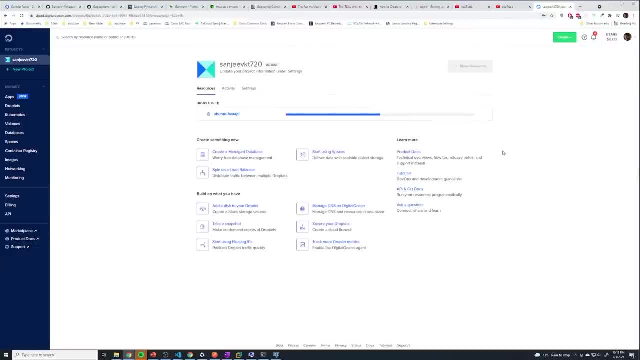 create our Ubuntu VM. All right, and once the loading bar finishes, you should see a public IP. this is the IP that we're going to use to connect to our virtual machine, And so we'll take a look at how to connect to this in the next video. 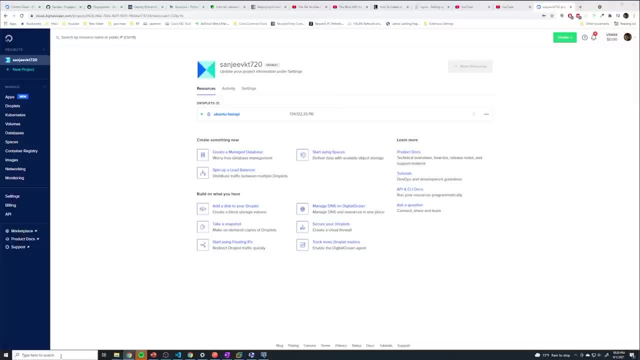 To connect to our Ubuntu virtual machine, we need to open up our terminal. So just search for terminal on Windows. If you're on Mac, you can do the same thing, just search for terminal And then on Windows you can select command prompt. 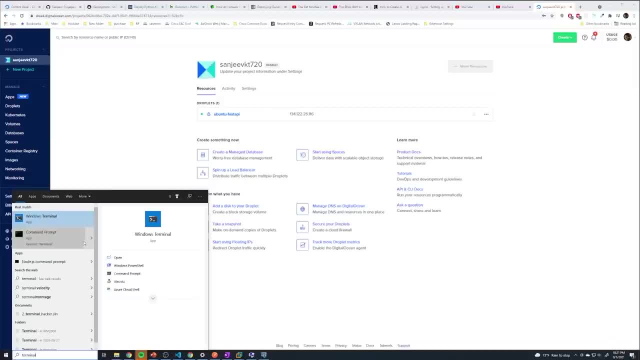 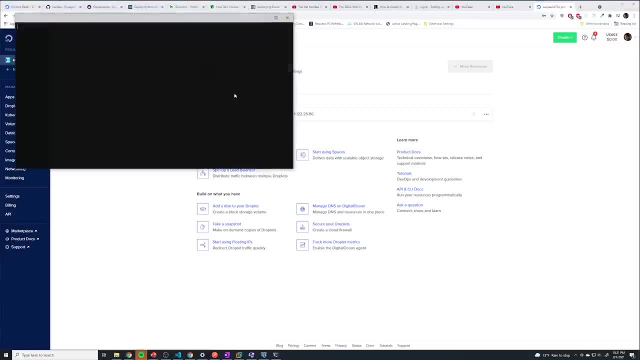 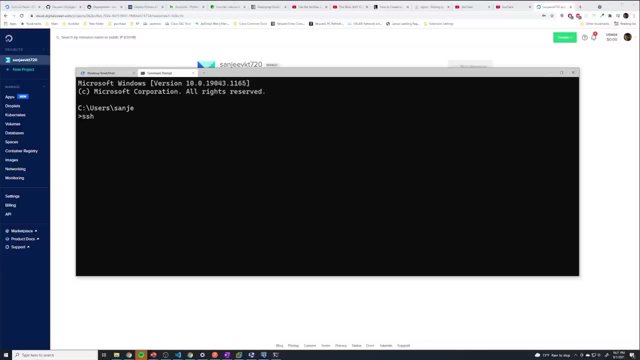 I installed another terminal, So I'm actually going to use that, But you can use this one as well. You can even use the built in terminal within VS code. it's all going to be the same thing. Okay, and to connect to a device, we have to use a protocol called SSH, So we do SSH. 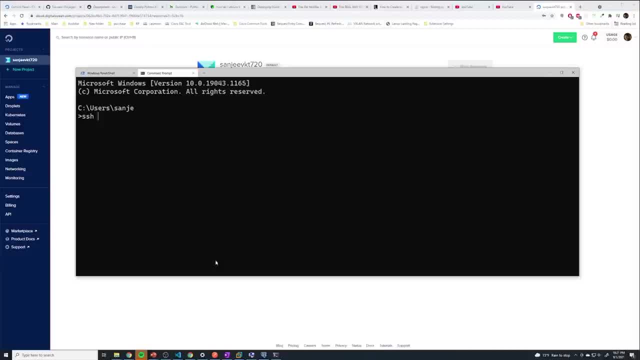 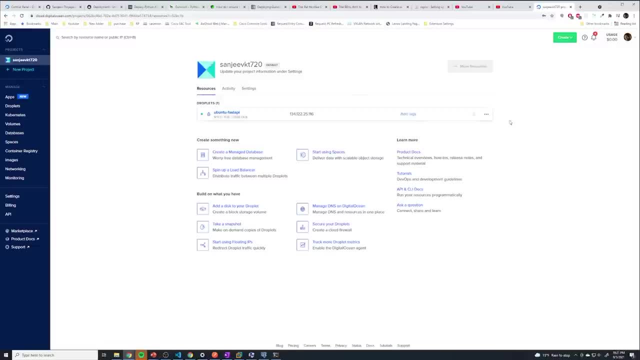 And then we have to provide the username that we want to connect to to the device, And so this is going to vary depending on where you're deploying your virtual machine. On DigitalOcean, this is, they're going to create an account for the root user, So this is like. 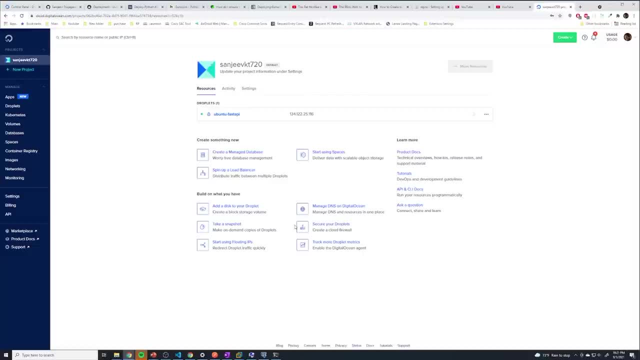 the most privileged user. this is where you can ultimately do anything with the device. you have unlimited access. So we're going to do SSH root at and then you do the at symbol And then we provide the IP address. So I can just 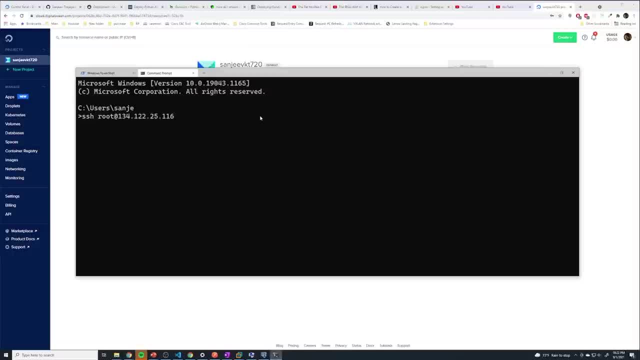 hover over this select copy and then paste it in here. At this point you'll get this- you know fingerprint message. So just hit Yes And then it's going to ask you for the password. So this is the password that we provided when we created the virtual machine. 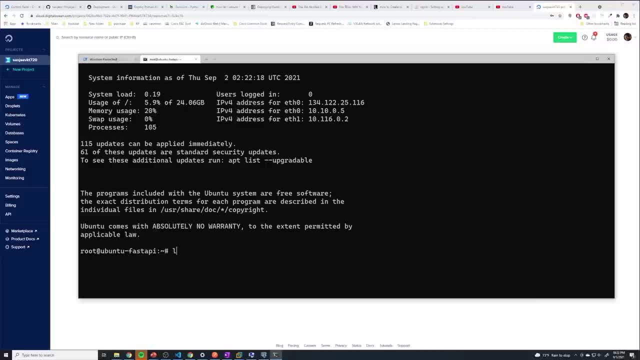 And at that point we are now successfully logged in And so you can be run LS. this is just going to print out the contents of your current directory, And so it looks like we've got one folder in our directory right here. But this is our Ubuntu virtual machine, And anytime you you get. 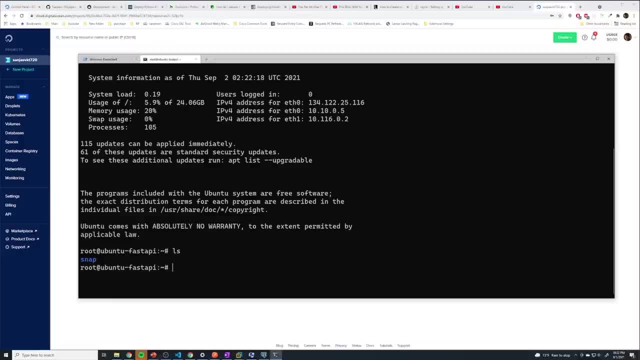 a brand new Ubuntu virtual machine. the first thing that we want to do is we want to update all of the installed packages. So we want to make sure that it's up to date, right, Just just like installing any other operating system. And to run that, there's two commands that we want to run. 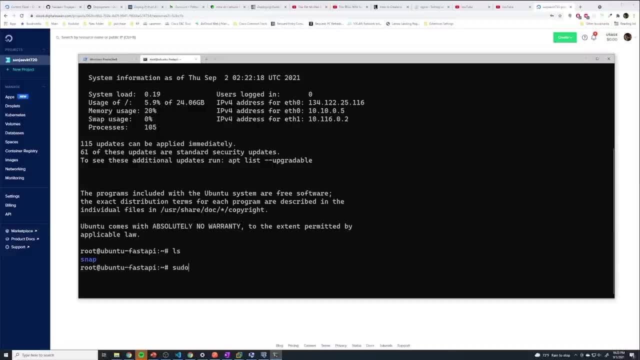 So we do sudo. So this is going to give you: well, technically we don't need to run sudo because we're the root user, But if, for some reason, you're not the root user, then you always have to use the keyword sudo. So we do sudo, And then we're going to run sudo, And then we're going to. 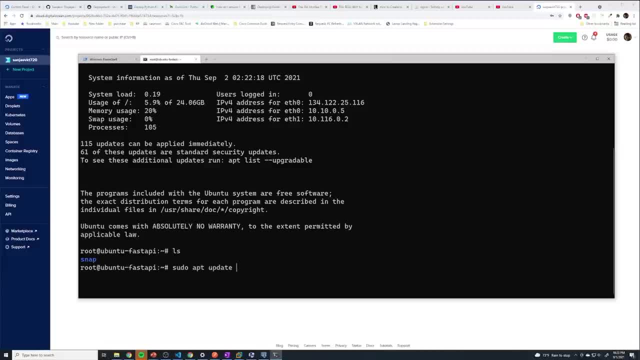 run sudo apt update And then the second command. we can do two- and signs and say sudo apt upgrade And then pass in a dash y flag. The reason we pass in the dash y flag is because if you don't pass in this flag, what's going to happen is it's going to do a few things and then a prompt. 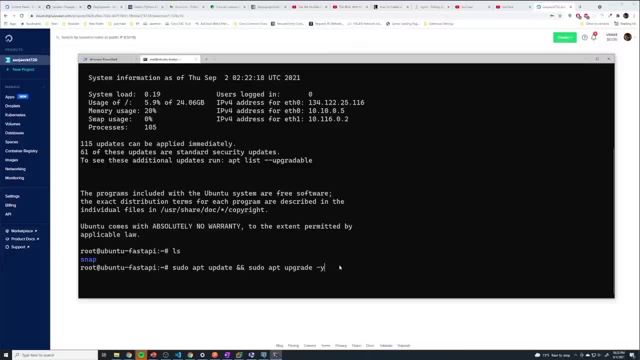 will come up or you actually have to hit Yes, And I always hate having to hit Yes when you pass in the dash y, you can let it run And then you can just go do something else, go get some coffee, because it is a fairly long process. 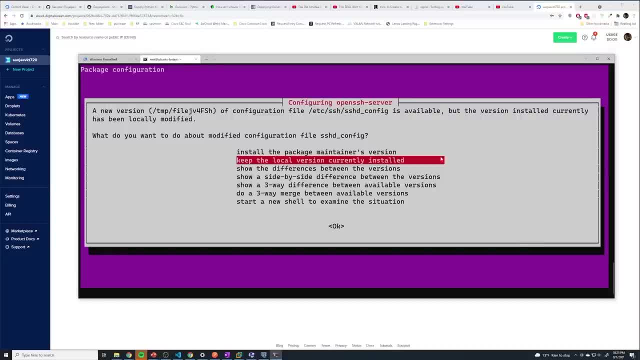 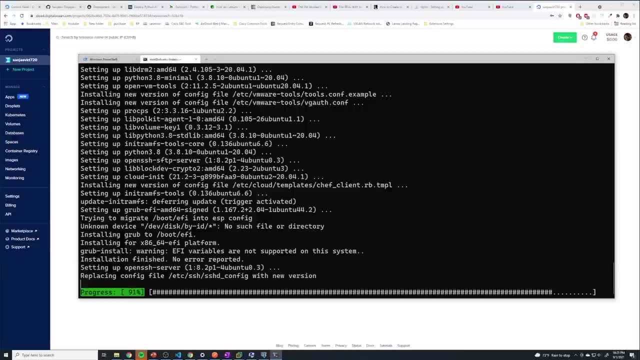 If you get this pop up, it doesn't really matter what option you choose. you can say: keep local version currently installed or install the package maintainers version. I'm going to select this one, but it shouldn't make a difference. So once all of those packages are up to date, we need to install. 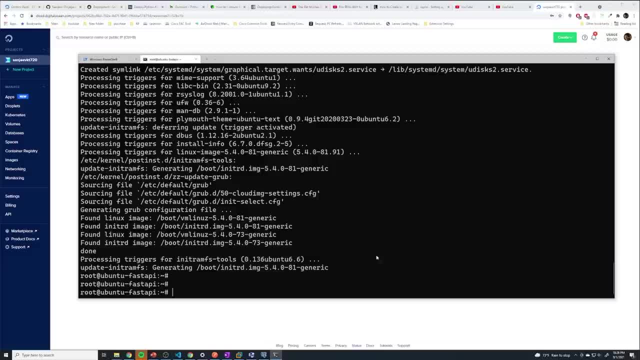 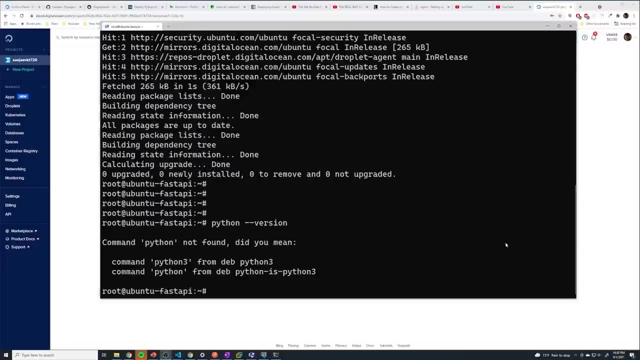 a couple of extra packages And the first thing that we need to do is: well, let's actually check what version of Python we're running on this machine. So, if I do Python, dash, dash version, alright, so it doesn't look like pythons installed. However, if I do a Python, 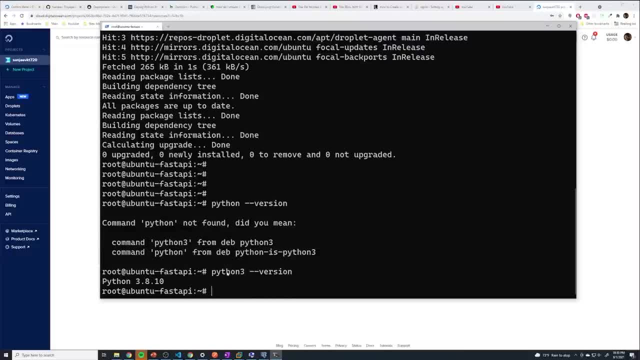 three, dash, dash version, we could see that we actually do have Python. it's just we have to use Python three because a version three of Python was installed, And so if you see anything that starts at 3.8.10, or later, you should be good. However, if you want to, you can always do a 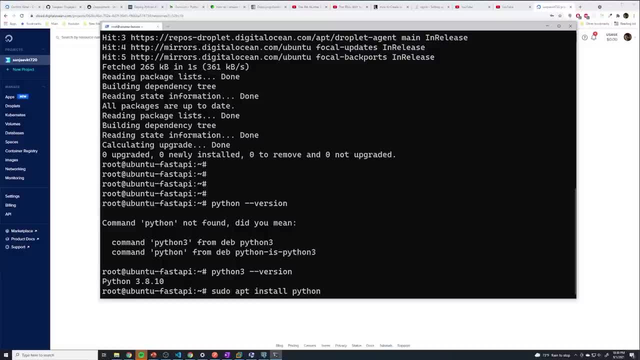 sudo apt install Python, And then I think you could just do a dash and specify the specific version that you want. But you can. you can figure out how to do that by taking a look at the Python documentation. 3.8.10 or later is better than 3.8.10.. 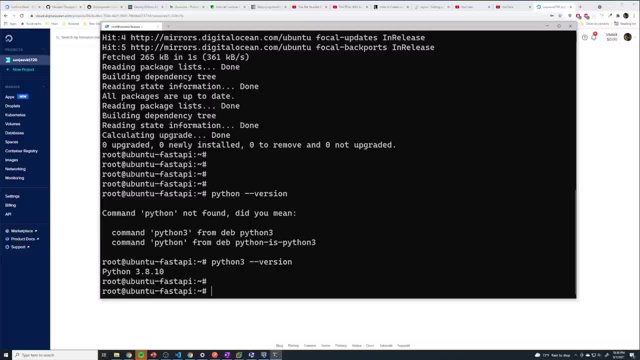 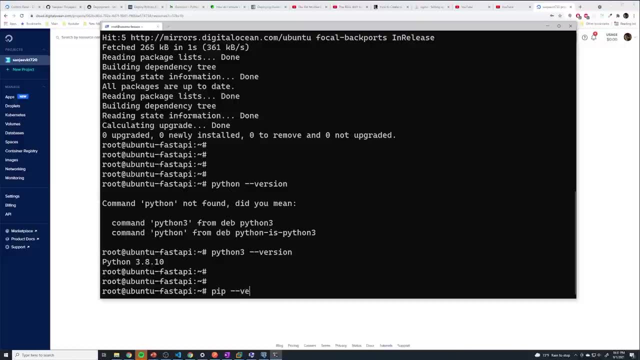 More than good enough for us. So we have Python. the next thing that we need to do is we need to install pip, And let's actually double check and make sure that it's not already installed on our machine. So we could just say: pip dash, dash version. We could see there's no pip here. 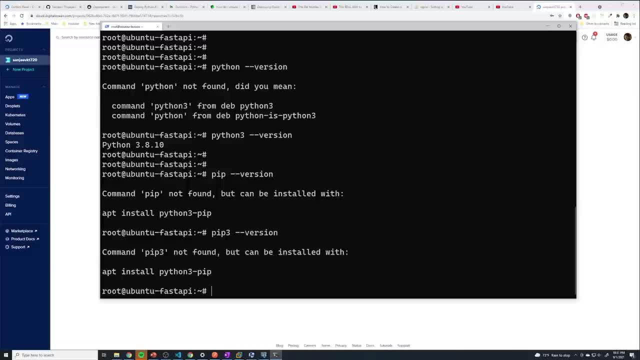 However, let's try a pip three dash dash version And it looks like we don't have pip installed. But it's giving us a little hint on how to install pip. So we can do sudo apt, install Python three dash pip And we'll hit Y. 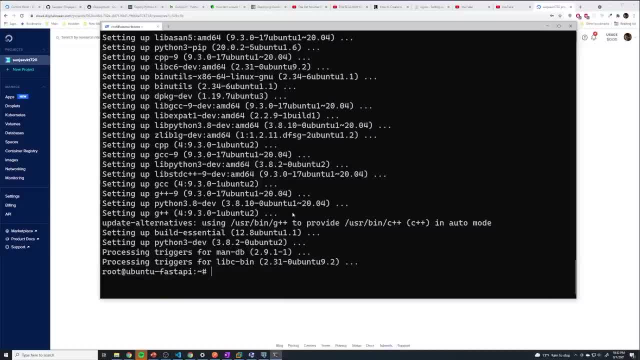 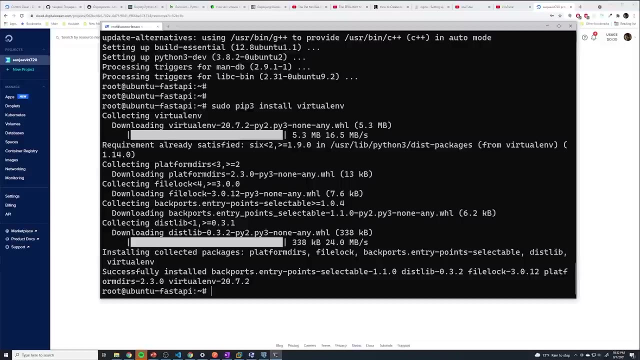 For Yes, And once that's done, we're going to use pip to actually install a virtual envy, because we are going to make use of virtual environments on this machine as well. So we'll say: sudo, pip three, install virtual envy, And so now we should be able to use the virtual environment command. 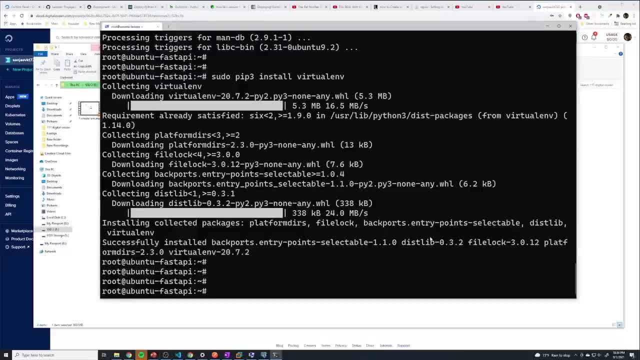 The next thing that we have to do is install Postgres on this machine, So we'll run sudo, apt install And then the libraries that we need, our post, grass ql and post for sql, dash contrib, And then we'll do a dash y so that we don't have to hit Yes. 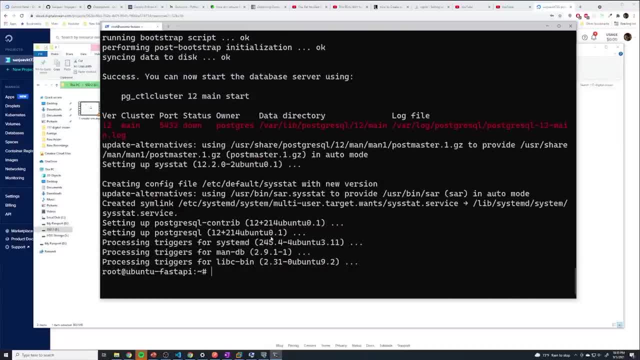 Okay, so we've got Postgres installed. How exactly do we connect to it? So what we're going to first do is, before we try to install it, we're going to go ahead and install it And then we're going to connect to it from our local machine. I want to connect to it from the actual Ubuntu computer. 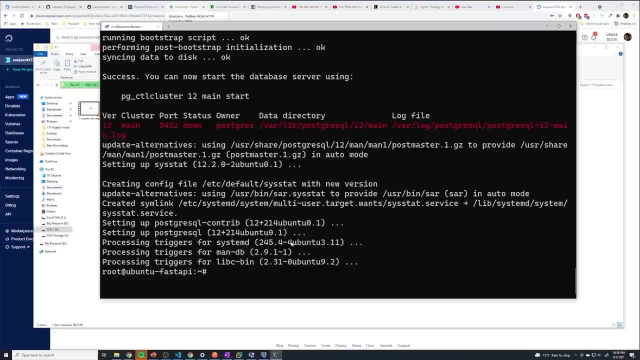 itself the Ubuntu virtual machine, And so we're actually going to take a look at the CLI for accessing the Postgres database, And so the tool that we use to do this through CLI is called PS ql Right, and we should be able to have access to it. So, if you do, PS ql, dash version. 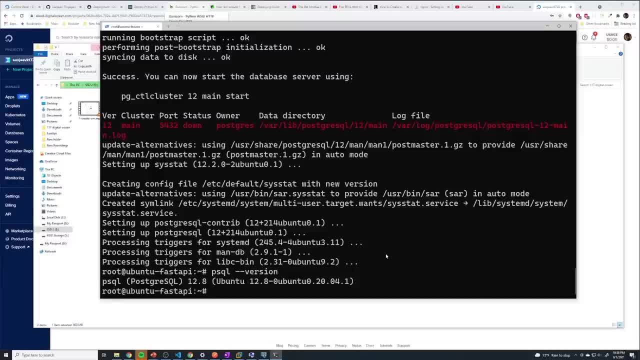 you should see that it should respond back with something. So that means PS Q L is installed And if I do a psql dash dash help, it's going to show that the virtual environment is not installed. if I do a psql dash dash help, it's going to show us the different flags that we can pass in. But 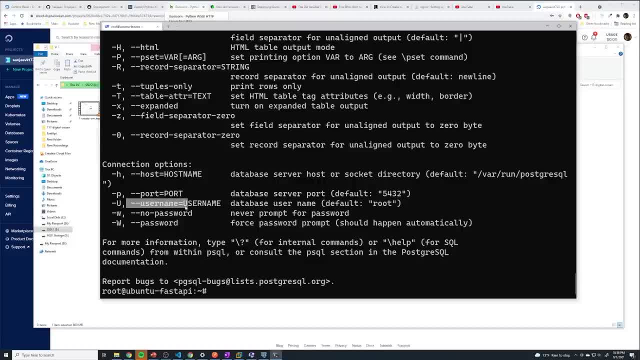 the main flag that we want to pass in is the dash us, so we can specify what's the username that we want to connect to. So let's say psql, then dash capital U and then our username. And we know that when we install Postgres it's going to install a user on the database called Postgres. 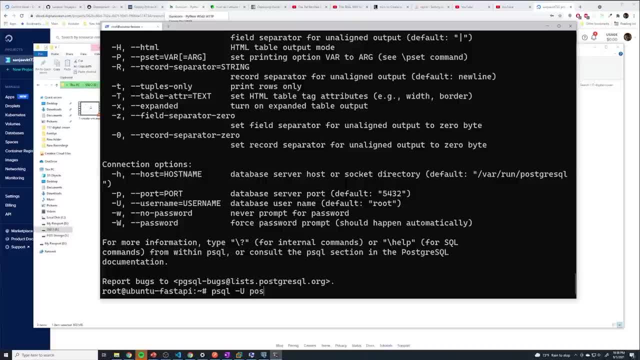 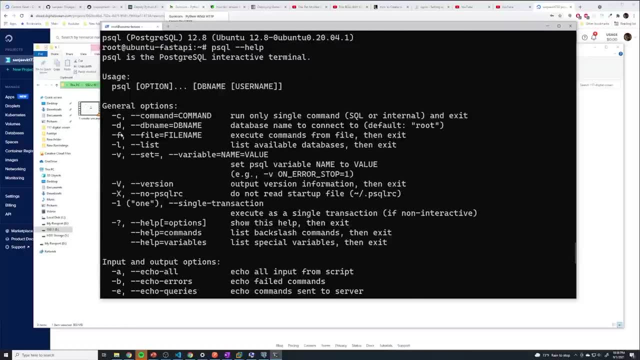 So that's what we always use to connect to it by default, And so we say Postgres. And if you want to, you can specify the specific database you want to connect to. that believe there's a flag. it might be dash D Yep, the database name. So you could technically say dash D Postgres. 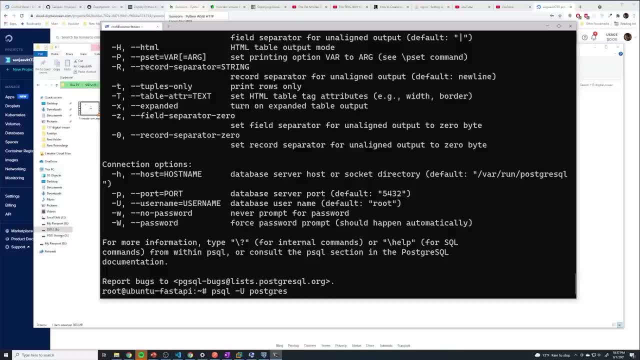 but Postgres is going to be the default, So you can leave that off And we're connecting to our localhost, which is going to be the default as well, So we don't need to pass in that, And the port we can also pass that in the default is 5432, which is what it's running on. 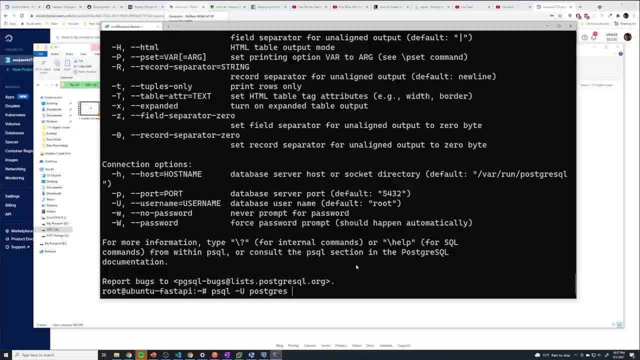 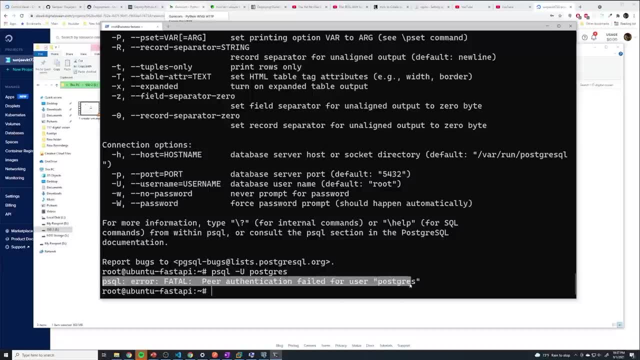 So we don't really have to touch anything else And we're going to try and connect like this. So let's see what happens. All right, and we get this error. it says a psql error: fatal peer authentication failed for user Postgres. So for some reason it's saying peer authentication failed And this: 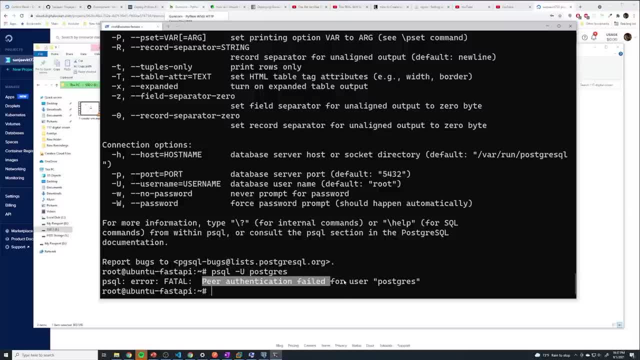 is a special meaning. right, It sounds like a regular login failure, but it's not, And it's because Postgres, when you install it on Ubuntu, it has a special way of authenticating users by default. So, when it comes to local authentication and what I mean by local authentication, 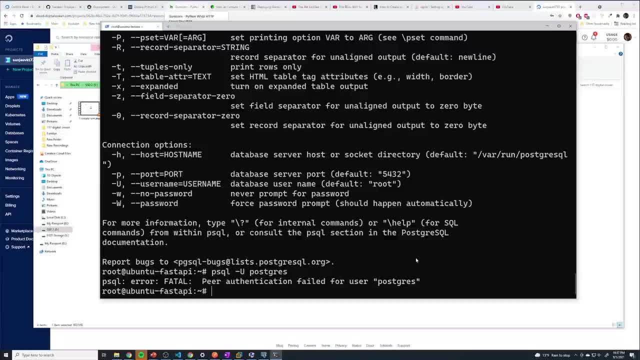 is the Ubuntu VM connecting to the database itself. That's what a local authentication means, Whereas if I'm connecting from my Windows machine to the Postgres database on this, on this Ubuntu VM that is not called, that is not considered local authentication. 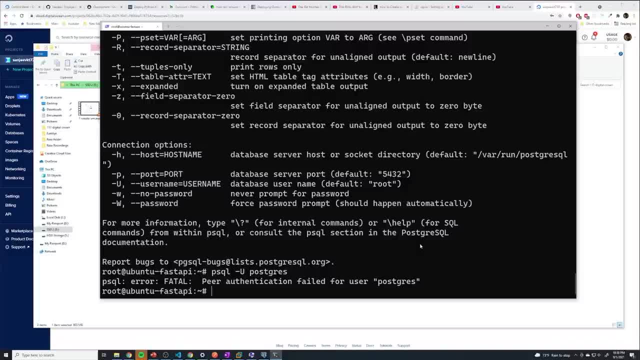 So, since we are on the same machine that we're trying to connect to our database, Postgres considers this a local authentication, And on Ubuntu, we have a special configuration called peer authentication. Now, this is the default configuration for Postgres. Now, this is the default configuration for Postgres. Now, this is the. 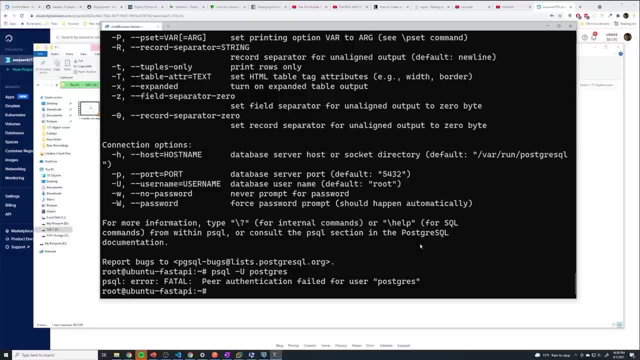 default configuration for Postgres And what peer authentication does is it actually takes the user that's logged in to the Ubuntu machine and it tries to log in as that user. essentially So, even though we pass in the dash u flag, since I am technically logged in as the root user. 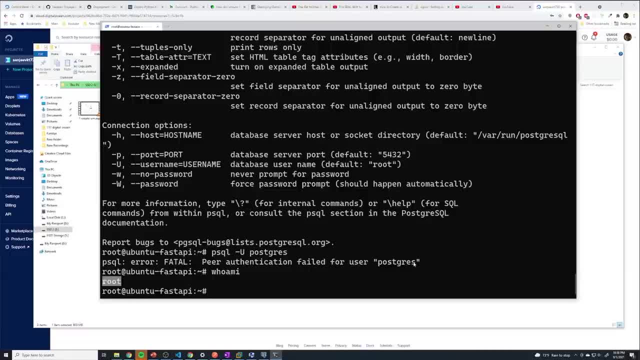 right, Postgres is going to error out because it will only allow a Ubuntu user called Postgres to be able to log in as the user called Postgres on the Postgres database. a little confusing, right, but it actually connects. it actually connects to the. 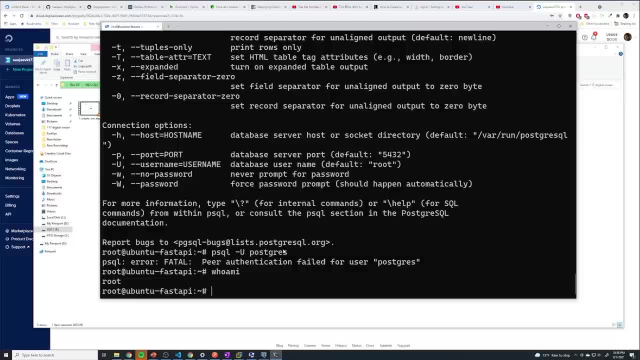 next, it actually obtains the username from the Linux kernel. So, whoever you're logged in as, that's the only person you can log in as, And so what we can do is, first of all, because this is the default configuration, Postgres understands that. so Postgres actually. 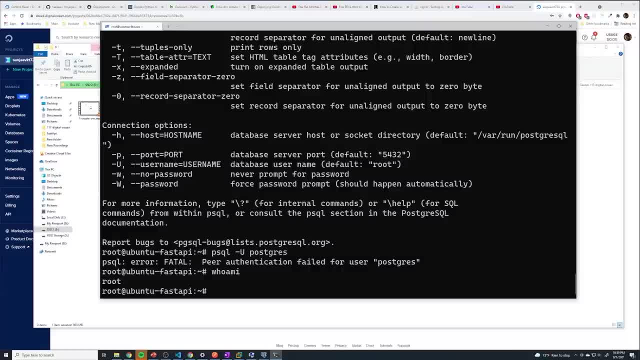 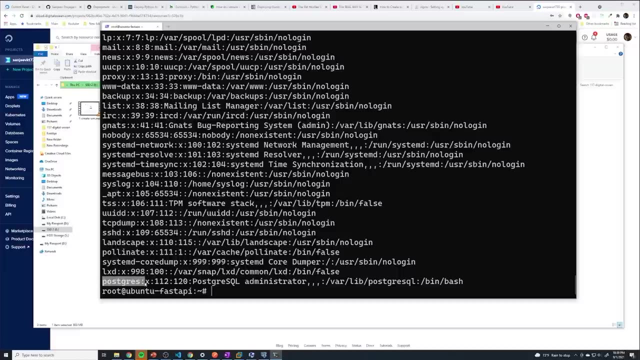 created a user on our Ubuntu VM called Postgres. So if you want to see the list of all the users on your Ubuntu machine, you can do a pseudo cat slash, Etsy, slash, path, WD And you can see all the users that have been installed And you can see that it actually created a user called Postgres. 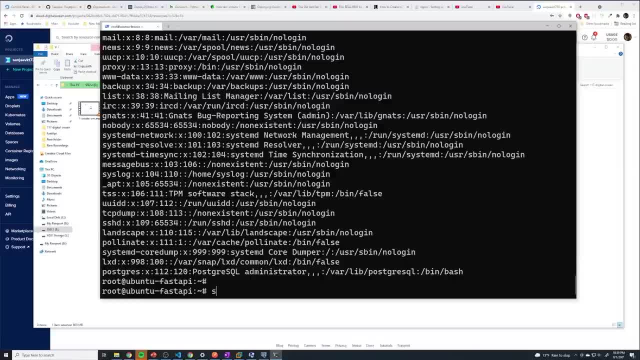 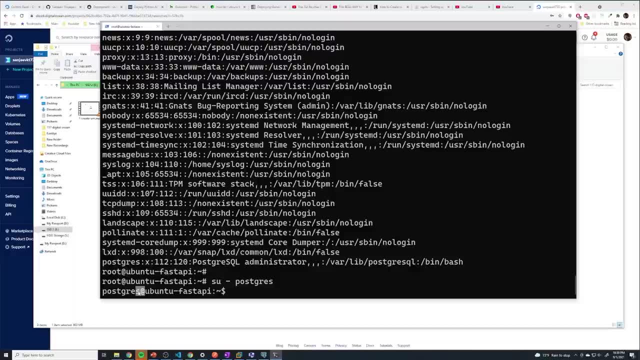 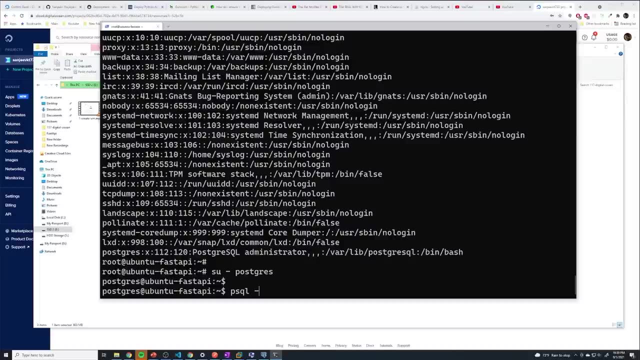 on this machine. So I'm going to change that user. So we can do that by doing sue dash and then the name of the user. So Postgres, right and notice how we changed to this specific user. And so now, if I try to do PSQL, dash u Postgres. 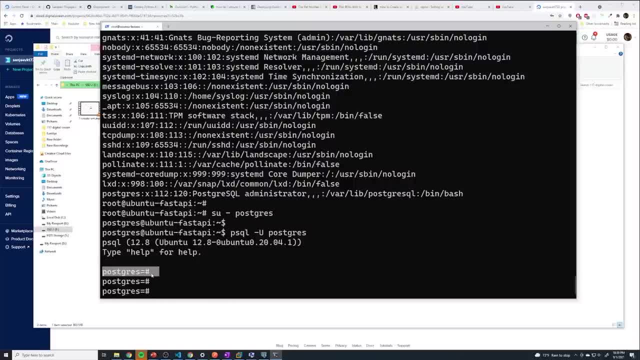 we can now log into the database. So if you see this, that means you're successfully logged in into the Postgres database. And while we're logged in here before we do anything else, because, first of all, we're going to get rid of that peer authentication, because I hate it- 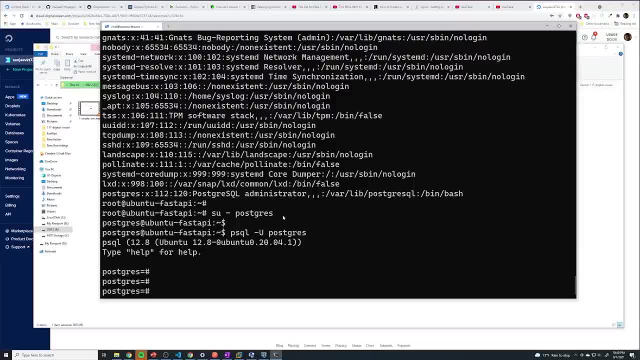 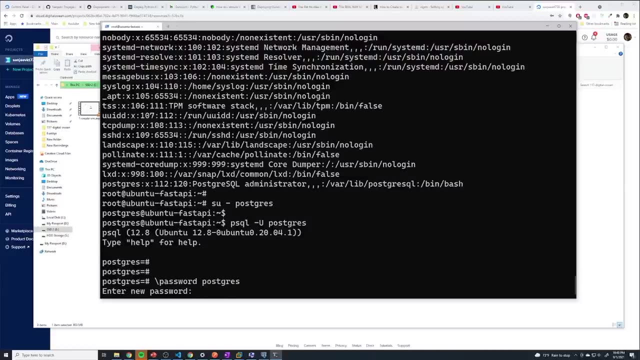 We want to create a password for our Postgres user And to assign a password to this user. we can say backslash: password and then the name of the user that we want to sign a password to. So we're going to use the Postgres user And then we're here, we're going to provide our password. 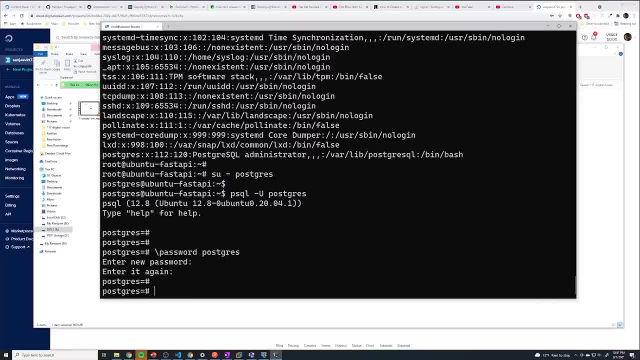 Alright, and so now we should have a password, And I'm going to exit out of here, So to exit out of the Postgres console or terminal, whatever you want to call it- you just do backslash and then Q for quit, And then we're. 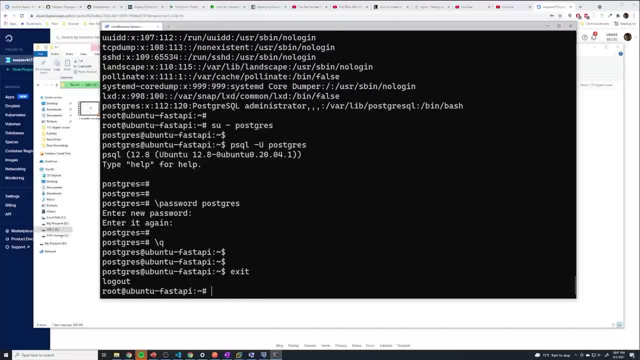 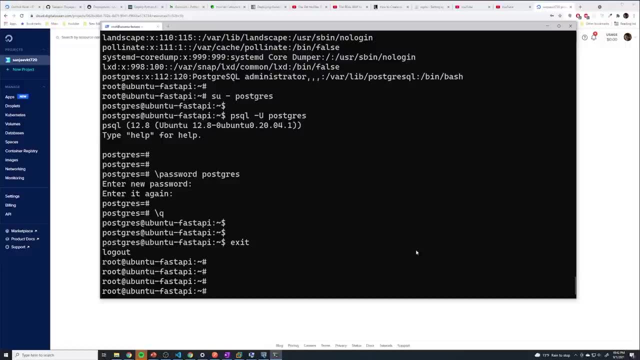 still logged in as the Postgres user, And so if you type in exit, it's going to take us back to the root user. There's going to be a few more things that I want to change to our Postgres installation, And so, anytime you want to modify the configs for Postgres, what we want to do is we want. 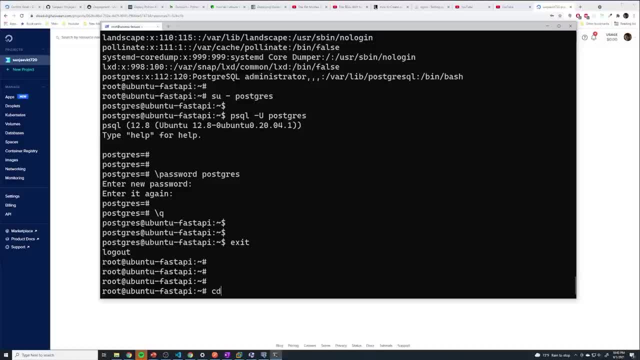 to move to a different directory. So the command to move to a different directory is CD, And then we specify the path, the directory. so we want to go to slash Etsy, So generally any application to install on Linux or Ubuntu machine, usually the configs for that. 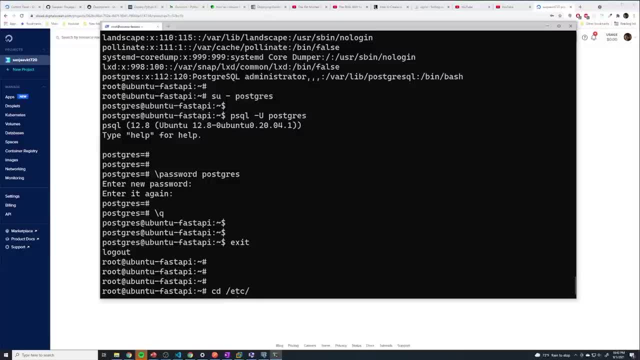 that package or that application is going to be in slash Etsy, And then here I'm going to say Postgres slash, And then if I hit tab, you can see that it's going to auto complete. So you're going to specify whatever version of Postgres you ran, And so in this case I have Postgres 12.. But 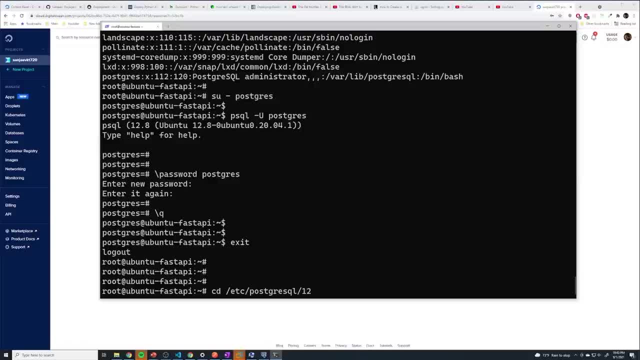 if you installed a version 13,, then you would put in: it would be a folder called 13.. And then you would put in a: it would be a folder called 13.. And then you would put in a: it would be a folder called 13.. 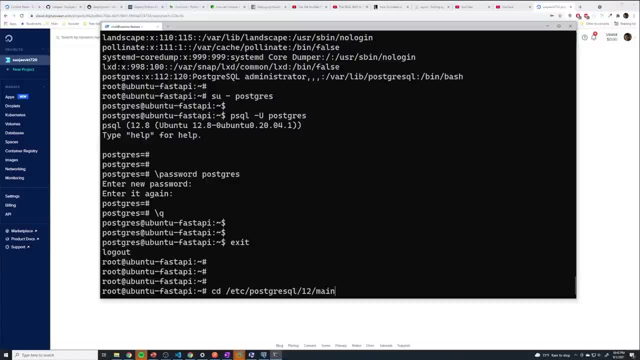 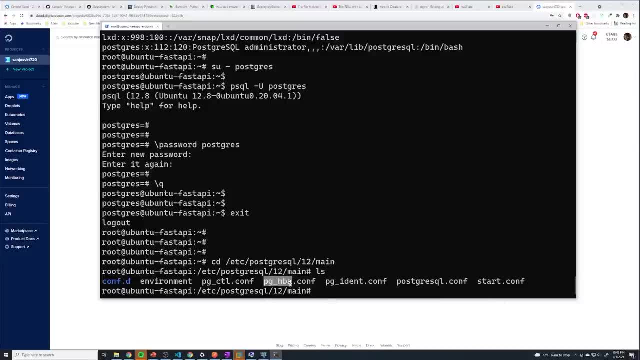 And then we will notice to main, if I type in LS, we'll see all of the files that we have in this folder And the two main files that we want to focus on, our PG underscore HPA, conf. So this is where we configure Postgres, as well as Postgres qlcom, And so we're going to open up Postgres. 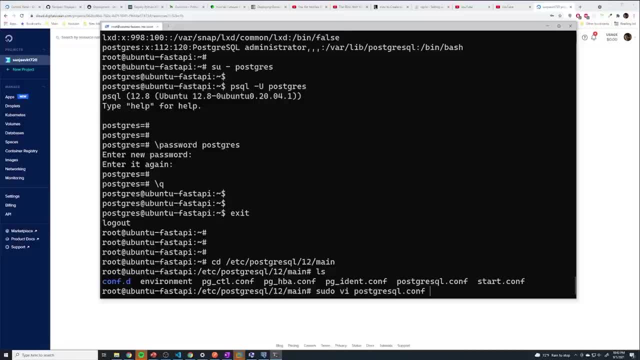 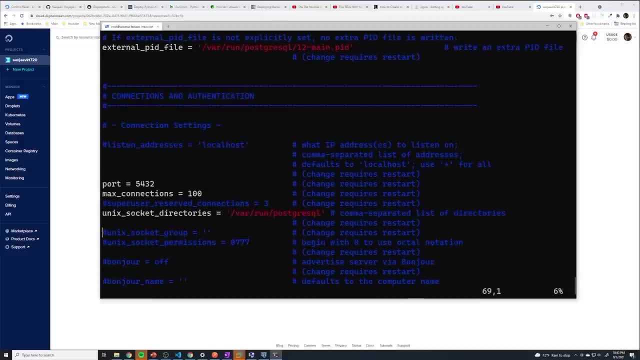 qlcom. So I'm going to say pseudo VI Postgres qlcom And we want to kind of scroll down And we want to take a look at the connections and authentication section, And so if you take a look at the default configuration, we can see that under listen. 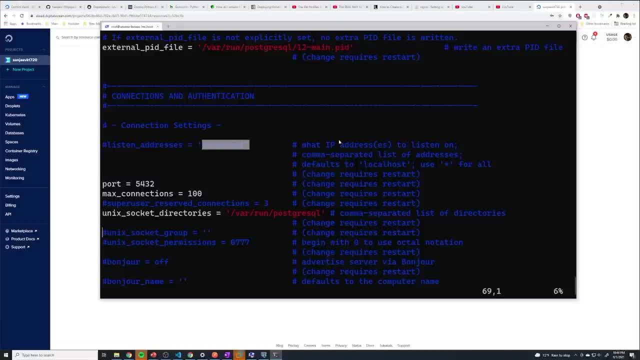 addresses. it's only going to allow localhost to connect to our database. That means only when we're logged into this Ubuntu VM can we then log in to this Postgres database. it is not going to allow me to take PG admin on my Windows machine and connect to it remotely. 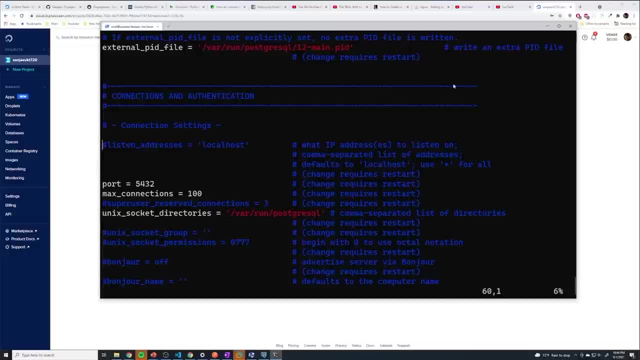 And so I want to change this. And technically you don't have to do this, But you know, if you do want to connect to it remotely, then you want to change these configs. And so I'm going to put this config. we're gonna say, listen, underscore addresses equals. And then here you would. 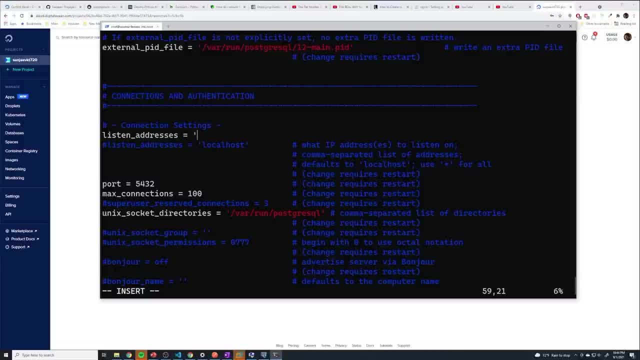 provide the IP addresses And so you know. if you wanted to only be able to connect to this database from you know, your, your office, then you would put the IP address or domain name of your office. If you want to allow all IP addresses to connect to it, you would just do a star. So that's what I'm going to do. 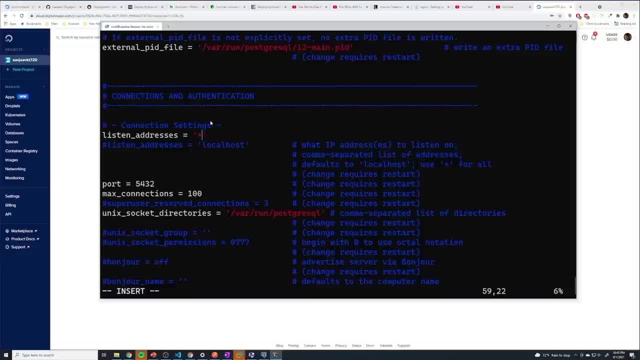 It's going to allow me to connect to this, regardless of what computer I'm on or where I am on the network. However, it generally, when it comes to best practices, you want to really narrow down the scope of the different IPs and domains that can access your. 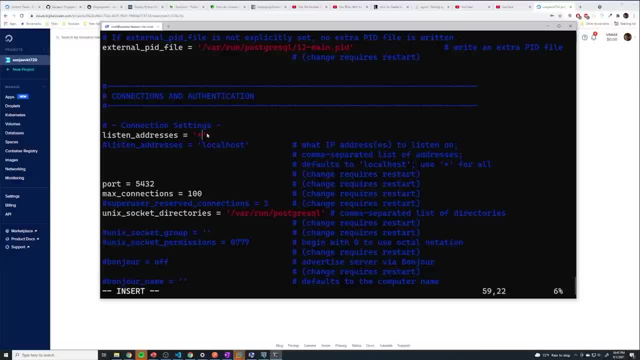 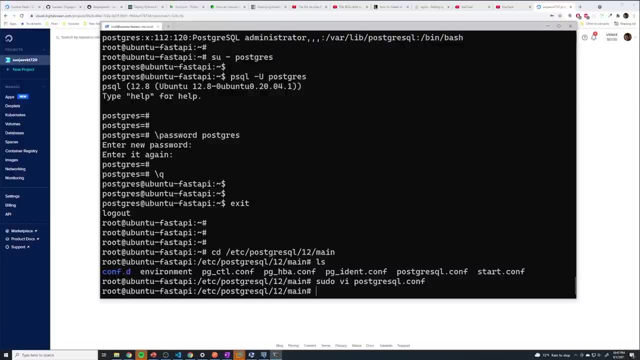 database, because that's the most important part of the application. you want to make sure it's as secure as possible. Alright, so we'll save this. that's the only change we need to make in this file. Then the next file that we need to change is PG, underscore HBA. 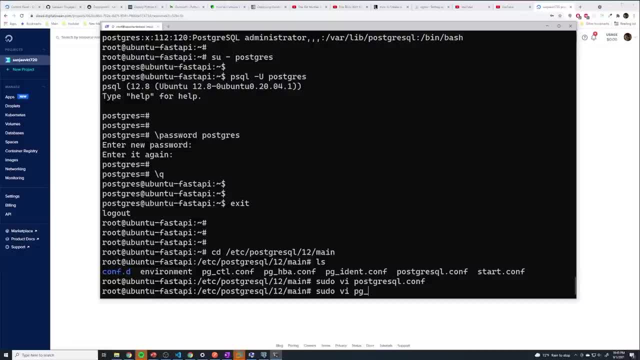 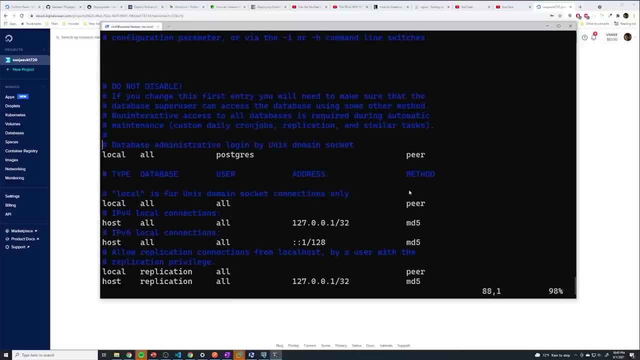 comp. So we'll do the same thing: sudo vi PG HBA comp And we're going to scroll down And we're going to take a look at our default configuration. So I did mention that when we connect locally it uses a peer authentication. So you can see that. 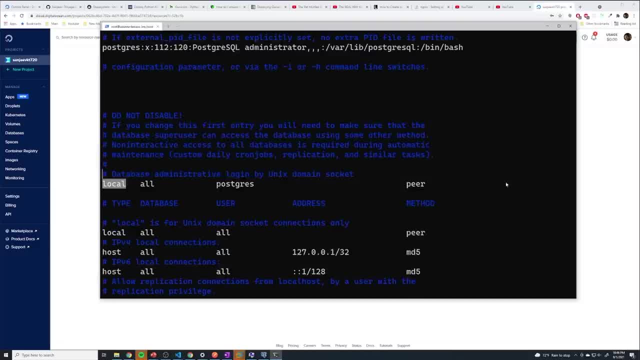 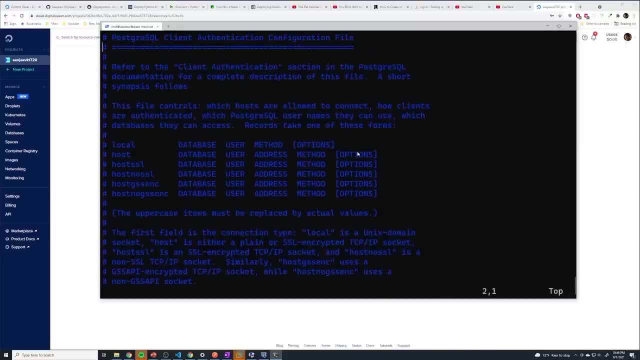 for local connections, And I forget what the second column is if we actually scroll up. I got to go up, Actually, let's see what the second column is. Okay, so this is going to be the format of it. So you can see that a случае to an IP address to a location. So we're going to 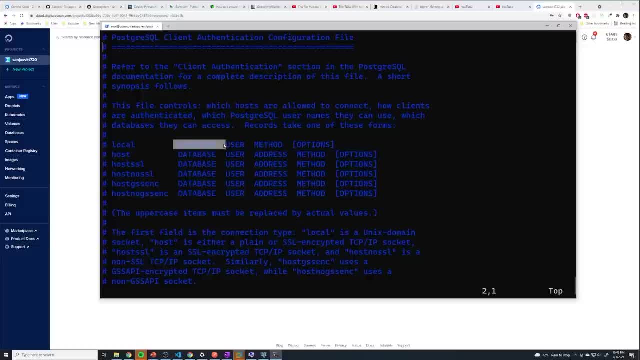 this is going to specify what type of connection, then what database this connection should be associated with, or this rule should be associated with what's the user and then what's the method. well, we also have address and method if you are connecting remotely, so we want to change this. so 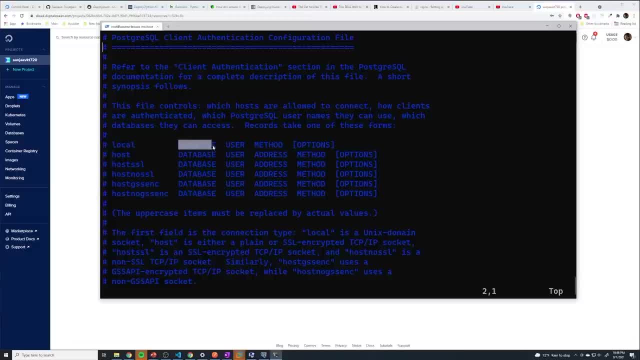 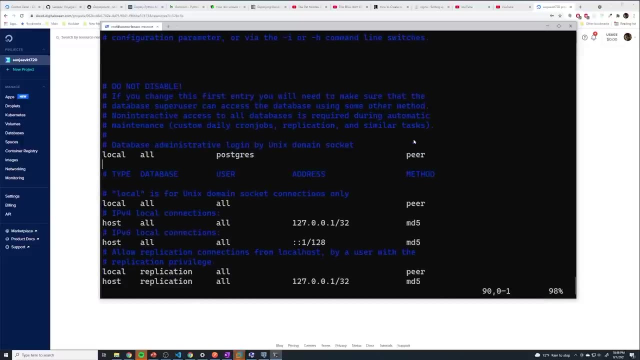 we want to say for local users, regardless of you know what database they connect to and what user they connect, as we want to make sure that we do not use peer authentication, we use regular password based authentication, which is md5 in this case. and so here we're just going. 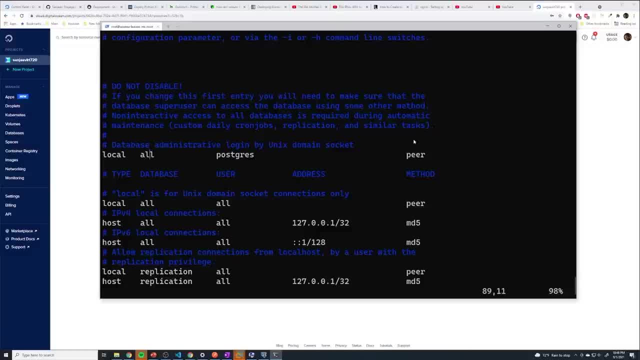 to change this. so this is saying, for any database, this rule is going to apply for the user postgres. we're going to say, instead of peer, we want md5, like we have here, so we'll say md5 so, and we're going to change this one to md5 as well. 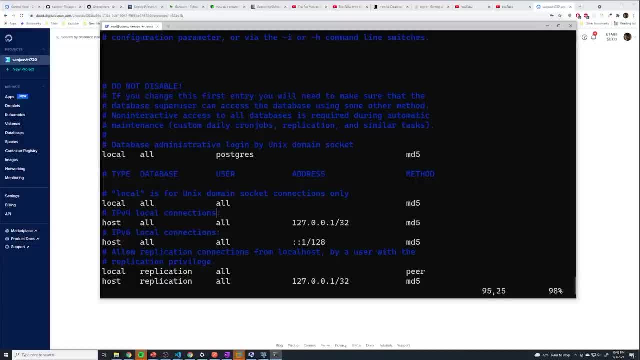 and then, lastly, for these two sections right here, these are going to be for remote connection. so if i want to connect from my windows machine, this is the rule that's going to apply. so this is saying that, for you know, hosts for any database, any user, right now the only ip addresses that can connect. 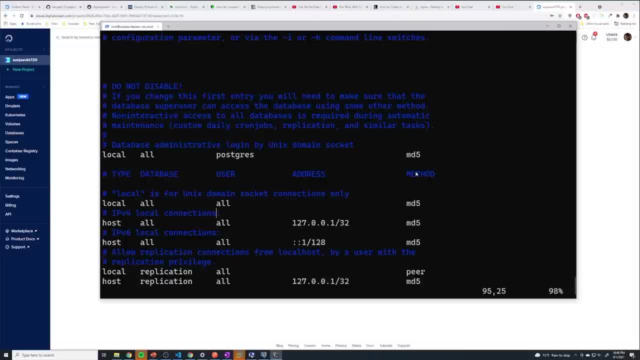 to it are going to be 127 001, which means local host. so that's effect effectively blocking all remote connections. so i'm going to go here and we are going to change this and i'm going to say 0.0.0 slash 0. so this means any ip address. 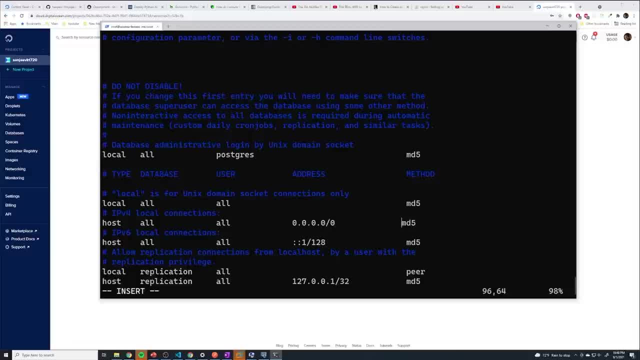 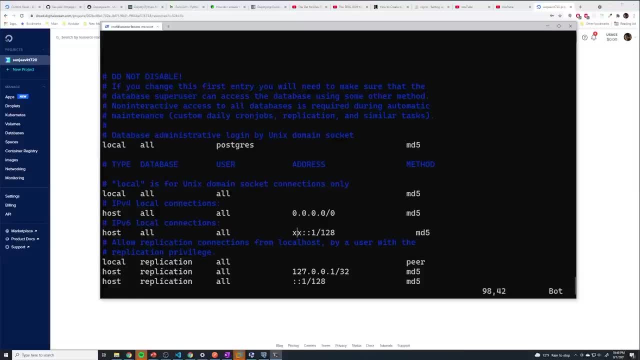 and then, just to keep things nicely formatted, i'm going to move that over there, and then we're going to do the same thing for ipv6, which is what this line is doing, and i'm going to say this: so this is the syntax in ipv6 for saying any ip address. 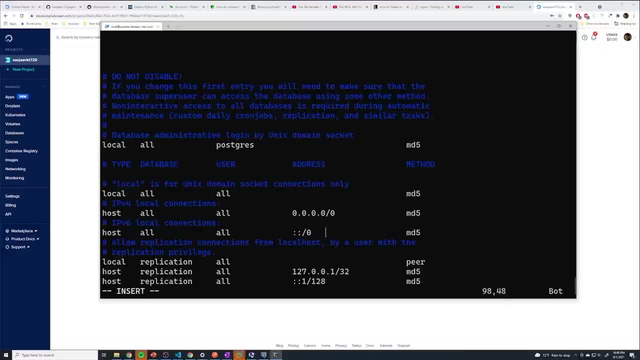 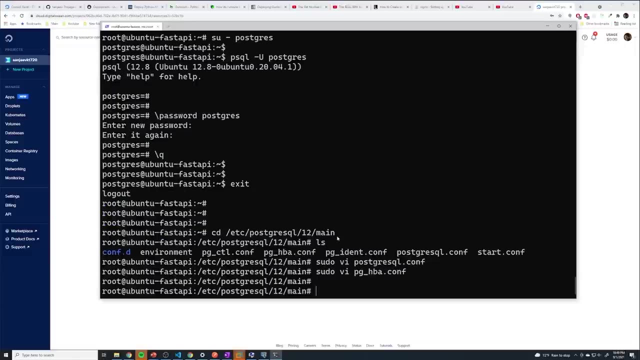 and that should be all of the config changes that we need to make, and so i'm going to exit out of here and make sure to save it all. right, and at this point, you probably think the changes have been made. however, generally, when you change any configuration file, you actually have to restart the application. 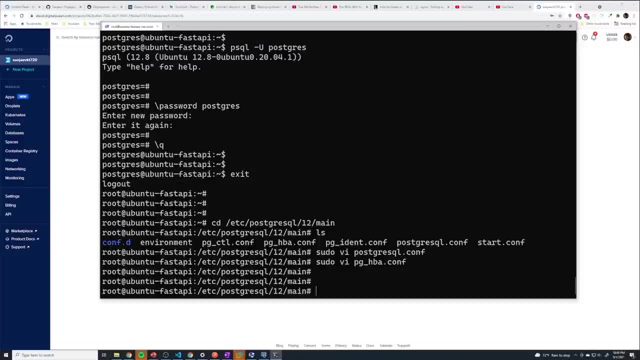 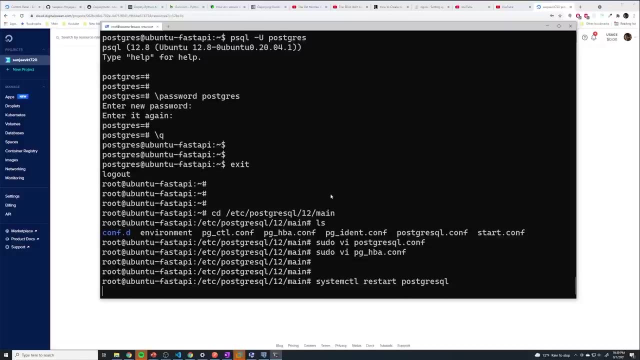 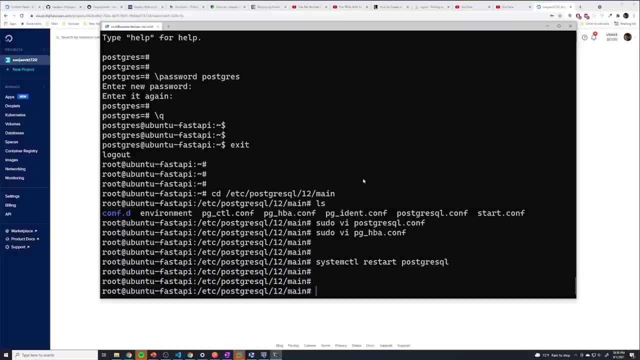 for the changes to take effect, and so to restart an application, you do system ctl, restart and then the name of the application. so this is going to be the name of the application. it's going to be postgres ql, all right, and it should be running at this point. so let's try this out now. 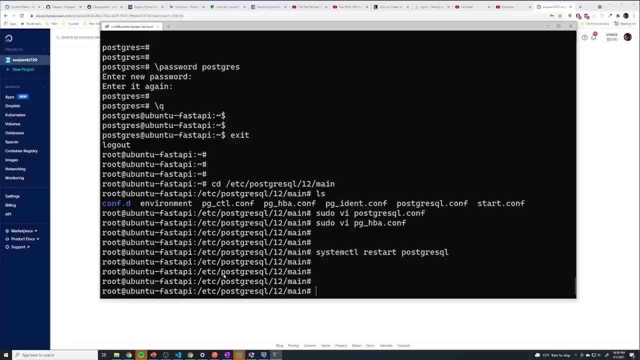 right now we are still logged in as the root user. so remember before we actually had to change to the postgres user on our ubuntu machine before we can log in as the postgres user. so now, instead, i'm going to do psql: dash u postgres and i want to see if i'm able to log in, and so now i actually get a prompt for a password. 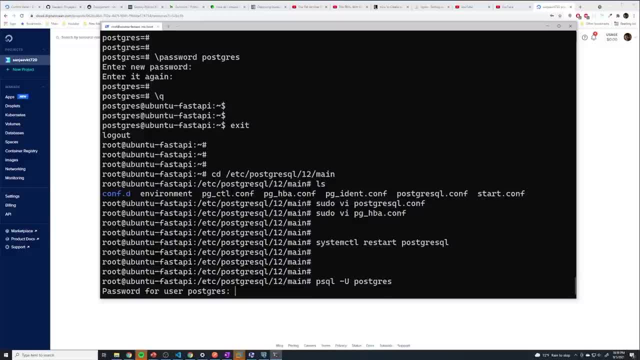 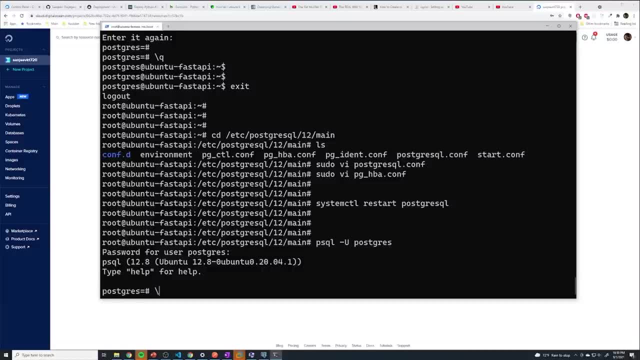 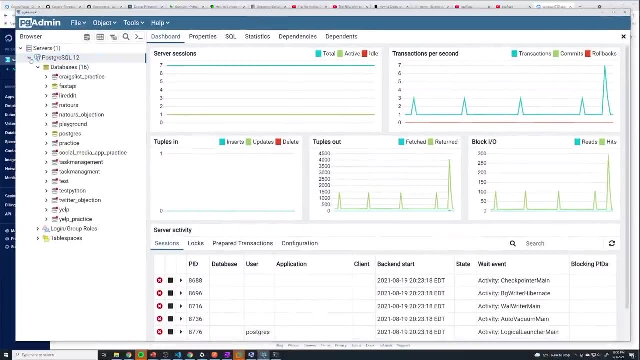 so it looks like things are working so far. so i'll try my password. and now we are successfully logged in to our postgres database. that's perfect. now let's actually try to connect to it using pg admin. and so pg admin, i've got my local machine, which is right here. 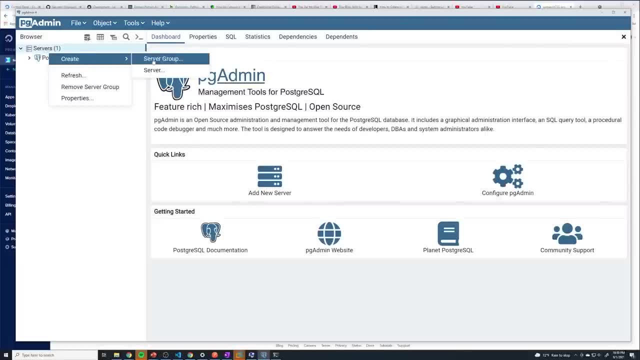 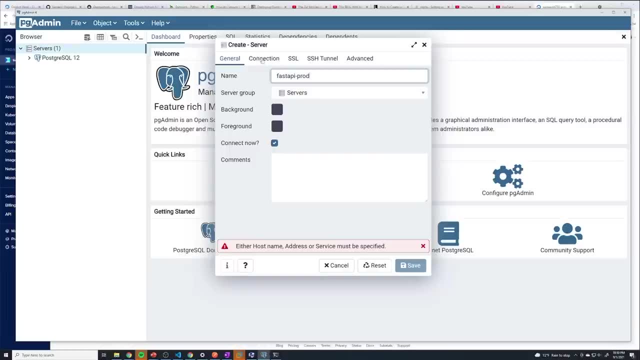 if i want to add a new machine, i'm going to right click on servers. we're going to select create server. give this a name. i'm going to call this fast api dash prod. call it whatever you want connection details here we're going to provide the ip address. 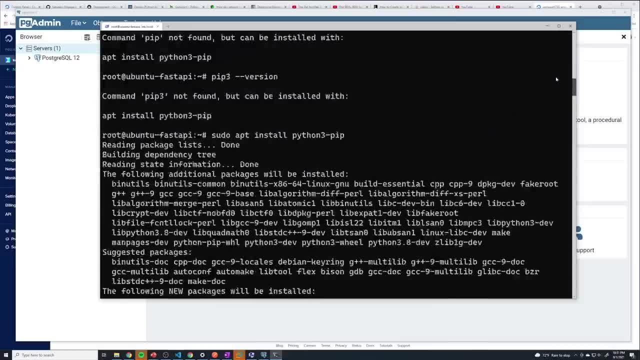 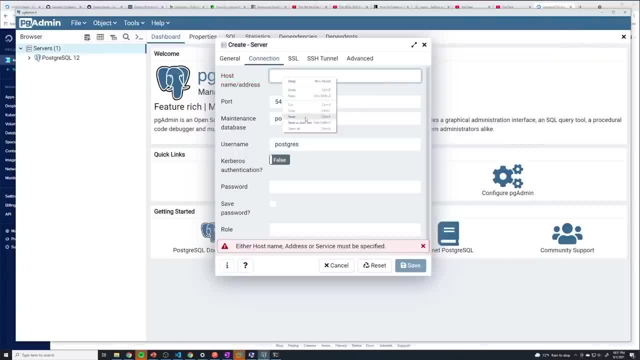 so i already forgot what's the ip address of our machine. we logged in one, three, four, one, two, two, whatever that is. we're going to provide this. that's the default port, that's the, the, the user we're going to connect as, and then, if we want to, we can put in a password here as well. 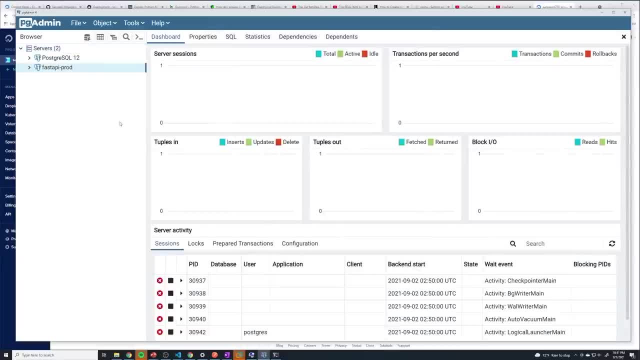 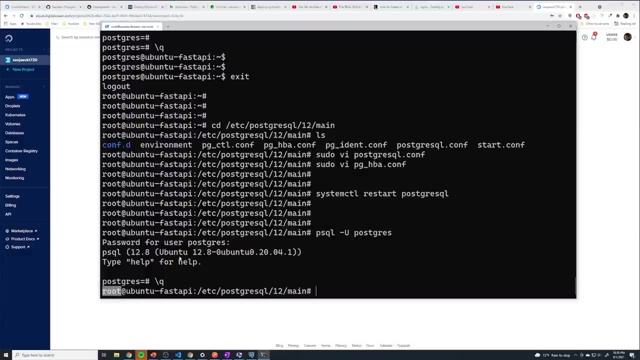 all right, and now we are successfully logged in to our production database. if i open this up, take a look at the databases. we just have the one default database that always gets installed. till now we've done everything as the root user and it's generally frowned upon in. 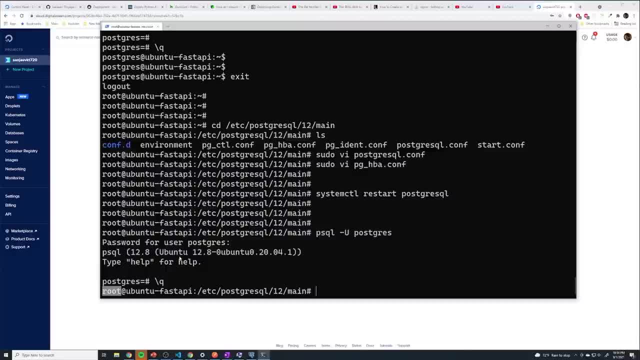 the linux world, regardless of what flavor of linux you're using- it could be ubuntu, centos, red hat- you generally don't want to be logged in as the root user because it opens the door for potential security vulnerabilities and it opens the door for the root user to be logged in. 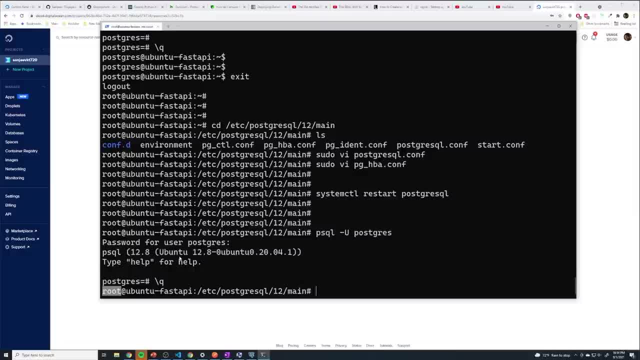 for you to potentially break your machine, and so what we're going to do is we're going to create another user. this user is going to have root privilege, so he'll still be able to make any of the changes, but it's better than being logged in as the root user and, more importantly, when we 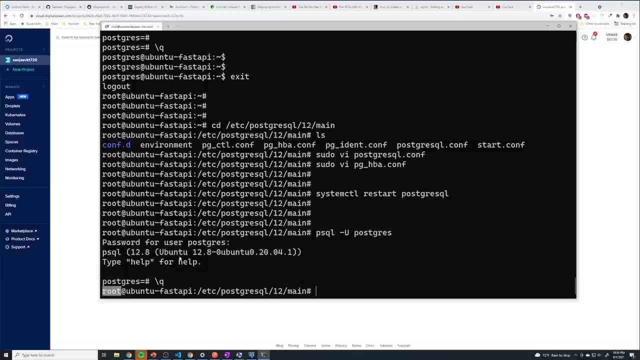 actually install our api, our python application, we're going to have our non-root user be the one responsible for starting it. we don't want the root user to start the application, because then we're giving our application root access to our machine and that is very risky. so instead we want a. 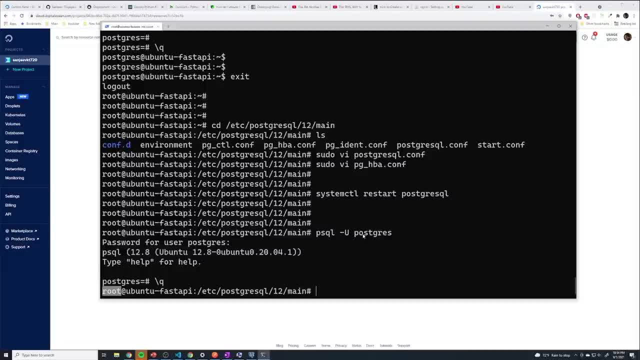 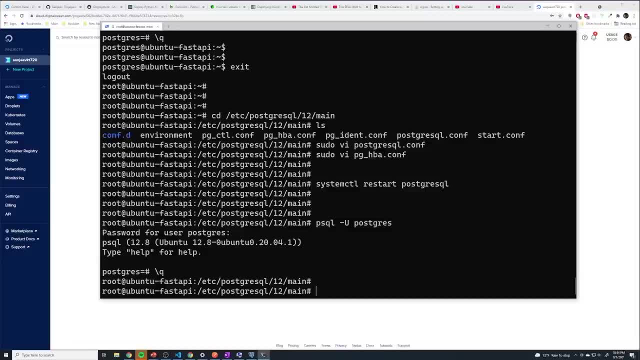 root user to start our api. so, on linux, to create a new user, you type in the command user mod- sorry, not user mod. we do add user and then the name of the user. so pick any name you want. i'm going to do sanjeev in this case, but you can name it like fast api or whatever you want. 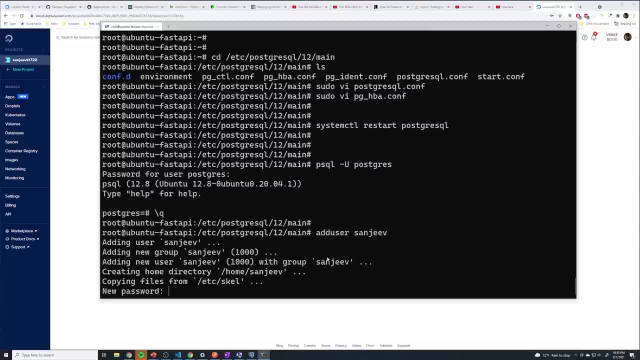 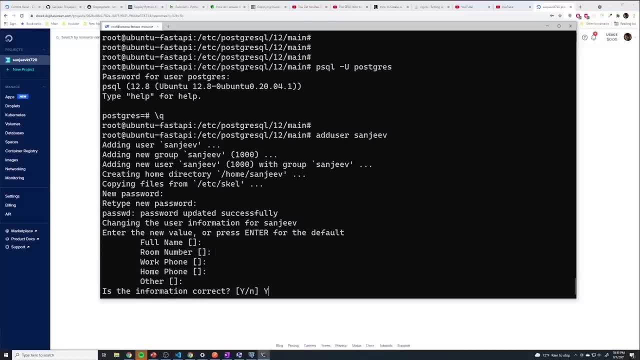 and then it's going to ask you for a password. so put whatever password you want, and then you can provide your name, and then you can add your username, and then you can add your username- but none of that really matters- and just hit y here, and so we've now created a user. 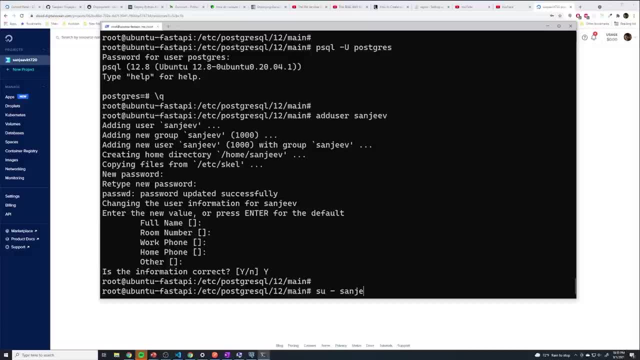 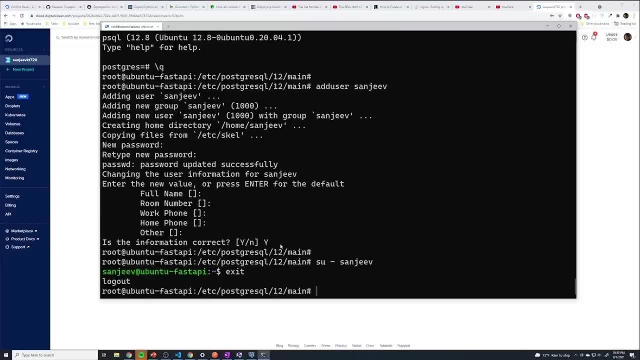 and what we can do is, if you want to, you can do a sue dash and then sanjeev, and then it's going to move you to the sanjeev user, or what you can do is you can exit out of this connection and then exit. 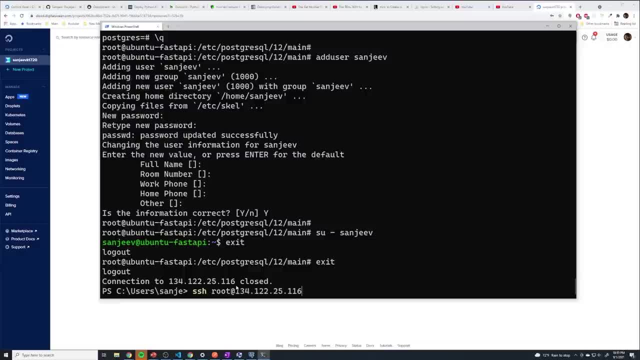 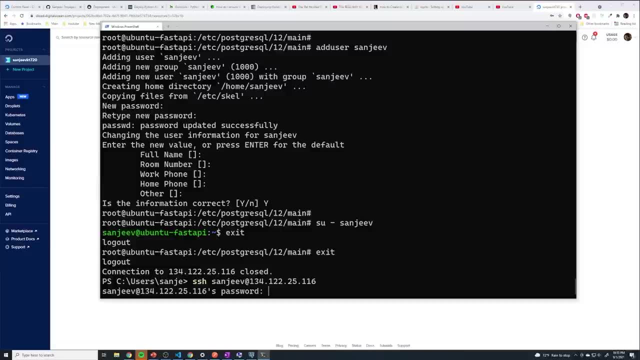 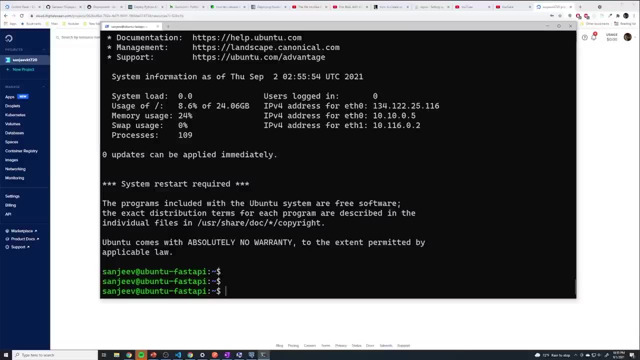 out of here altogether. so now we're back on our local machine and instead of when you do an ssh root to add whatever, you can change this to the new user that you just created, and so that's going to log you in directly as that user. now this user by default doesn't have root access. so if i try to do, 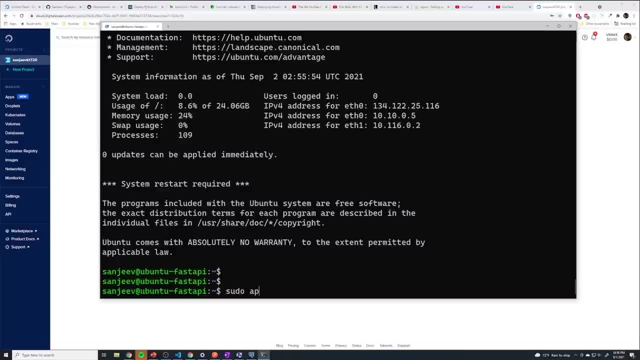 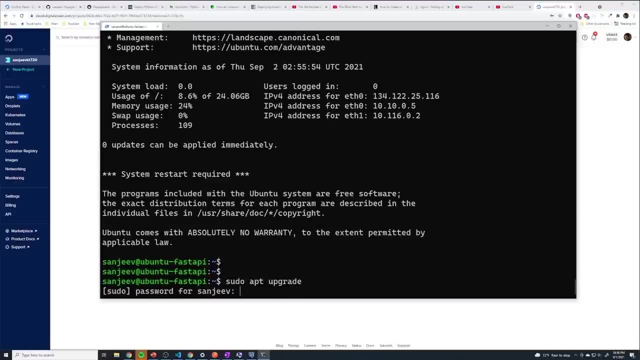 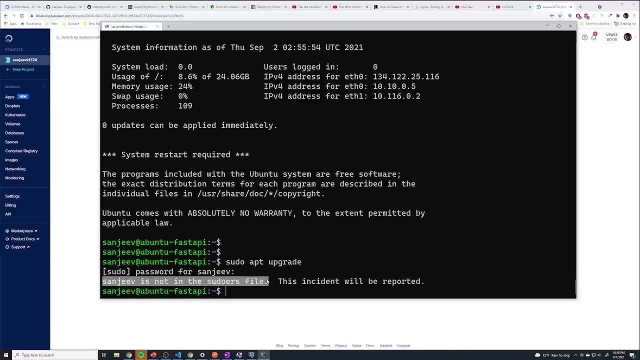 um, you know sudo apt upgrade. right, it's going to ask for sudo password for sanjeev and i'll put my password in and take a look at the error that we get. it says sanjeev is not in the sudoers file. this incident will be reported. so anytime you create a user, you have to give him. 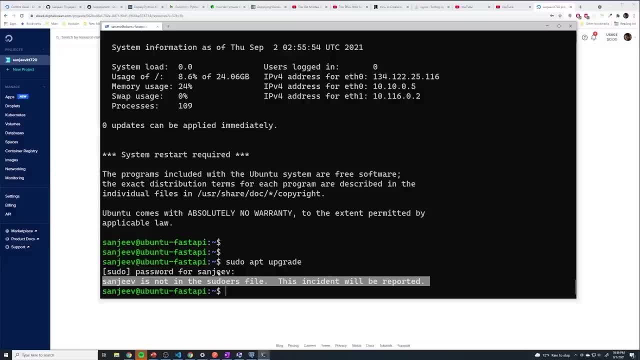 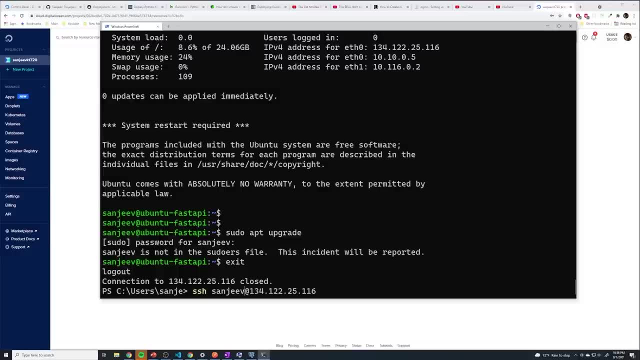 sudo access or root access to the user and then you can do that. so i'm going to do that here: root access so that he can actually perform operations that require root privilege. so we're going to have to exit out of here once again. i'm going to log back in as the root user. 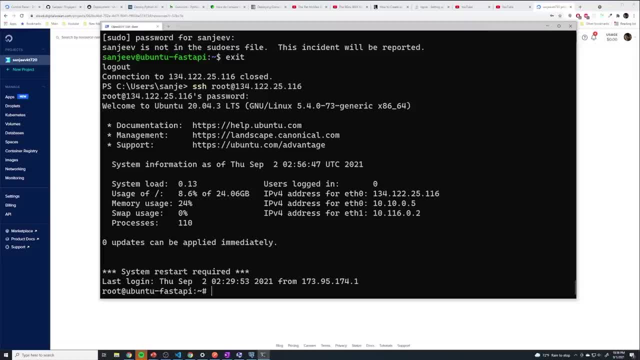 and to give a user root access, we you run the command user mod and then we pass in the flag dash a and then capital g- make sure it's capital- and we say sudo and then the name of the user. so i created a user named sanjeev, so i'll just put that in and so at this point, the user sanjeev. 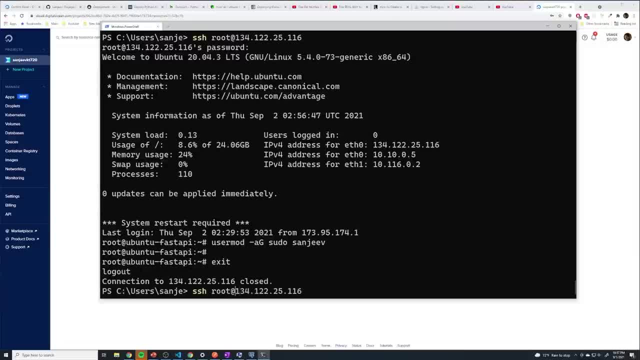 has a root access. so i'm going to log back in as the root user and then we pass in the flag as root access. so let me exit out of here again and we're going to connect back as the user sanjeev. and so now i'm going to run sudo, apt, upgrade and so, if i try that, put my password in. you can see. 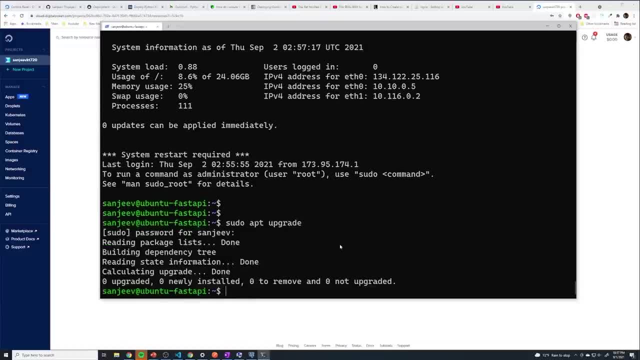 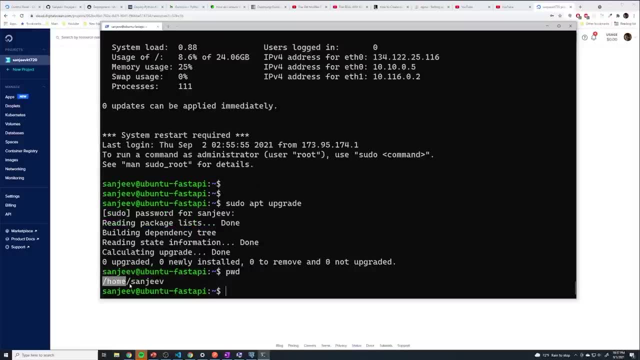 the command run, so we now successfully have root access. if you type in pwd, this is going to tell you the exact directory that you're in. so i'm in a folder called slash home- slash sanjeev. so whatever your user name is, you're going to be able to access the root access. so i'm going to. 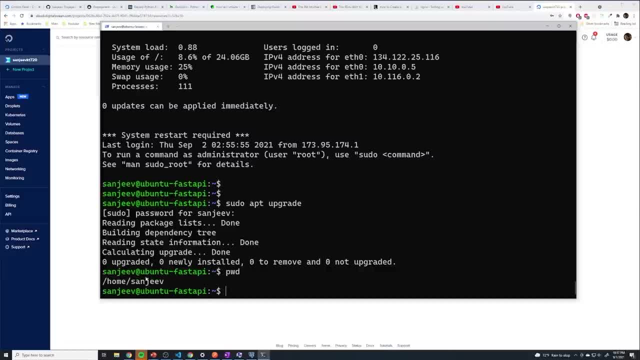 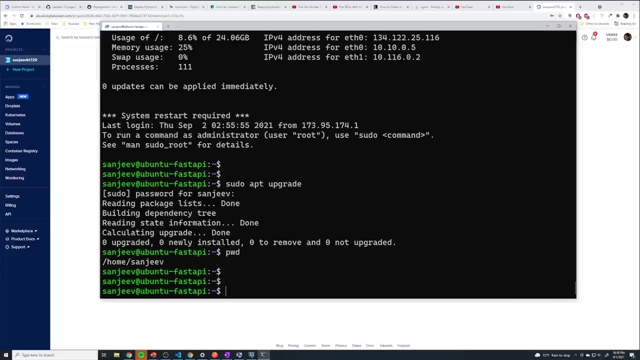 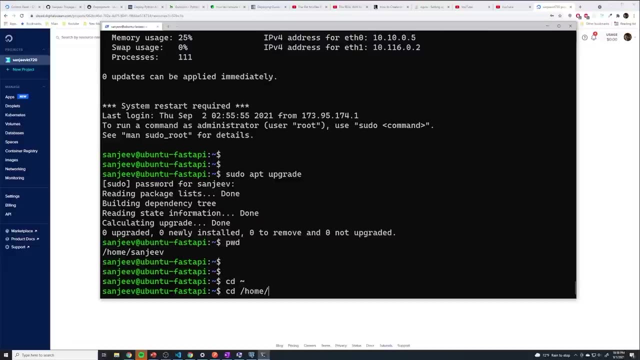 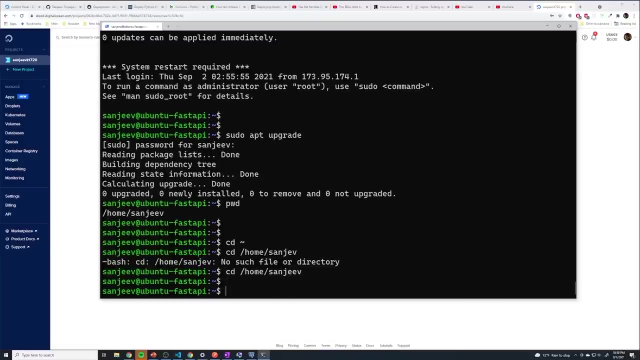 go ahead and say cd, and then it's going to take you to your home directory. or you can do cd, slash home and then your username that's going to take you here. whoops, all right. so once you're in your home directory, what we're going to do is we're going to create a folder for our application. 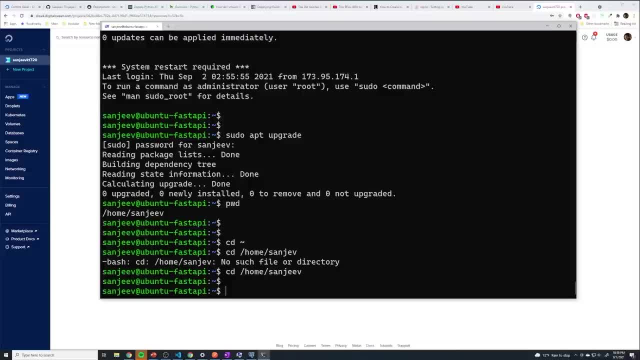 technically, you can put this anywhere on your machine. i'm just going to put it in my home directory, and then i'm going to put it in my home directory, and then i'm going to put it in my home. So I'm going to call this this folder app, or we could call it fast API doesn't really. 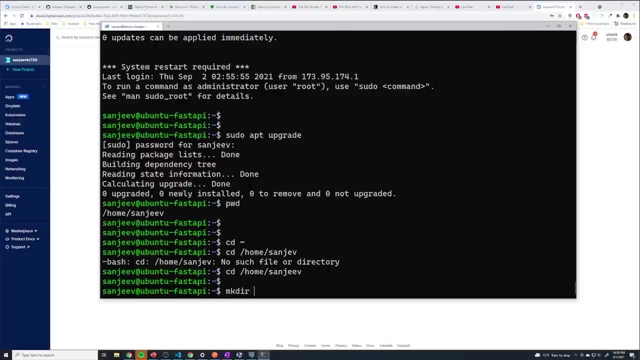 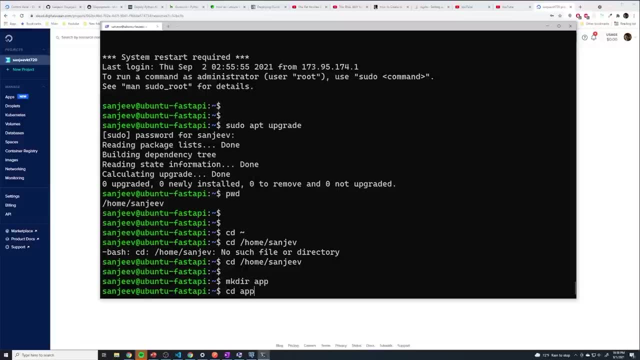 matter, They'll say mkdir. This is the command to create an app- sorry, create a directory- I call this app- And then to move into that app. we do CD app And within this folder, what we're going to do is just like we did on our local machine. 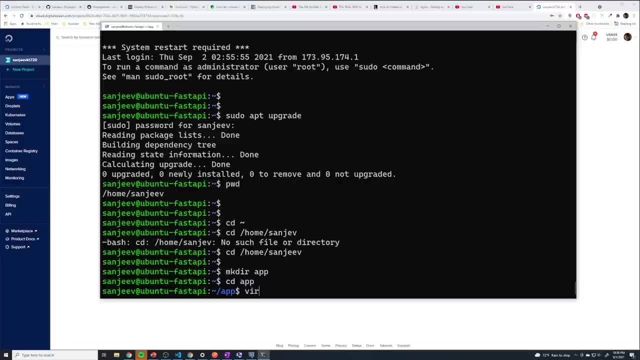 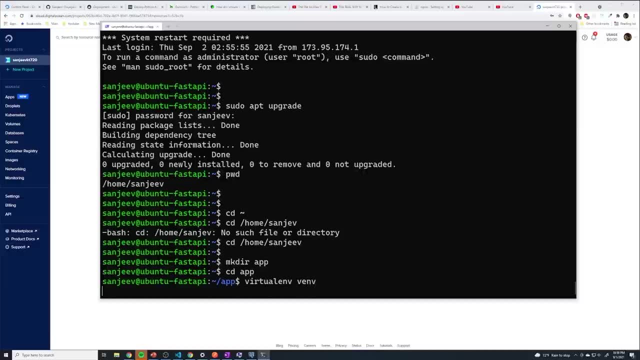 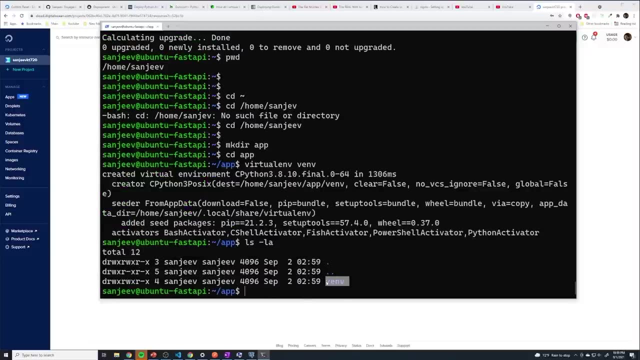 we're going to create a virtual environment, So I'm going to say virtual envy, And then we'll call our virtual environment V and V, All right. and then if I do an LS minus la, let's just make sure I created the virtual envy folder. then, to activate our 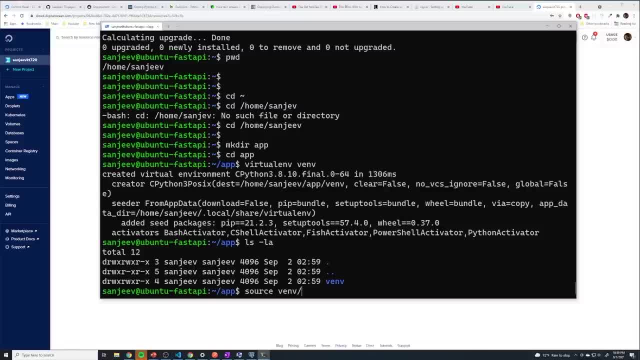 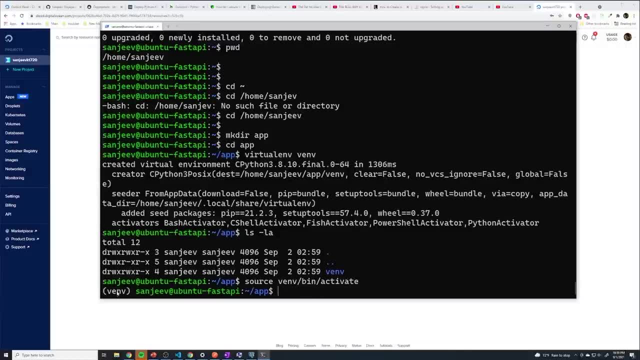 virtual environment. we'll type in the command source And we go into the that folder, the bin folder and then the activate file. Alright, and then we should see this little nugget right here. So this is going to let us know that we are currently in a virtual environment. 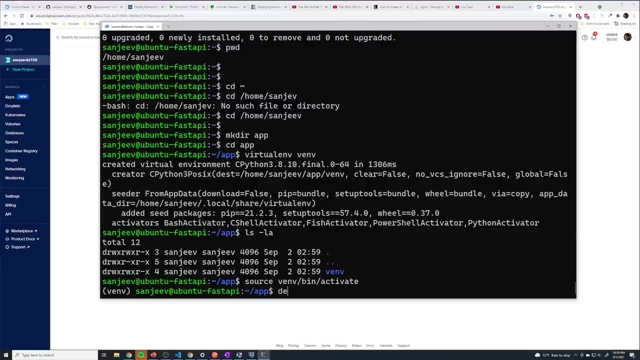 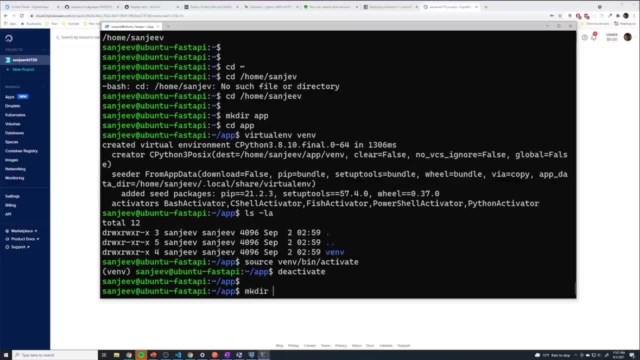 And if you ever want to get out of the virtual environment, you can just say deactivate. Within our app directory we're going to create another folder called source. So this is going to contain all of our source code. So we'll CD into the source. 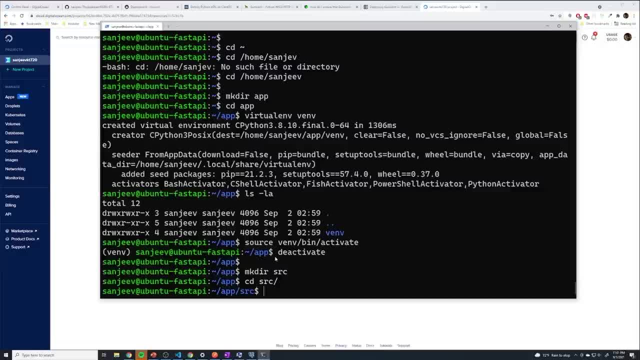 And now what we're going to do is we're going to copy all of our code onto this machine. And so how do we do that? Well, since we already have it stored on GitHub, all we have to do is just go to the URL for. 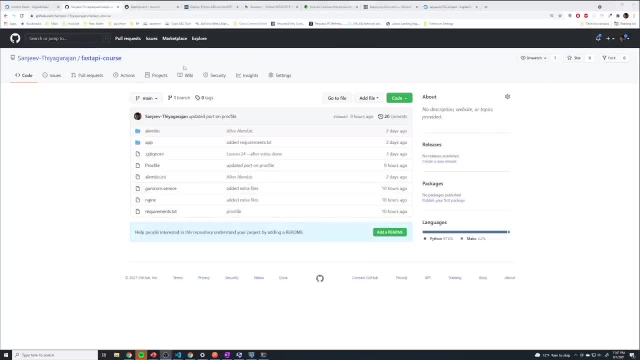 our app. We're going to go to our repository, So this is my repository that I created. This is the main one called fast API dash. course, This is public, So any of you guys can access this, but you're going to go to your specific repository. 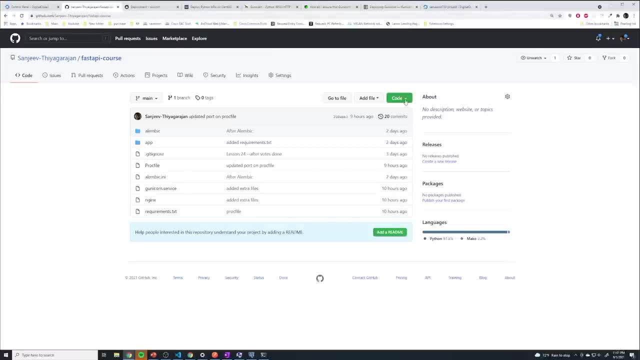 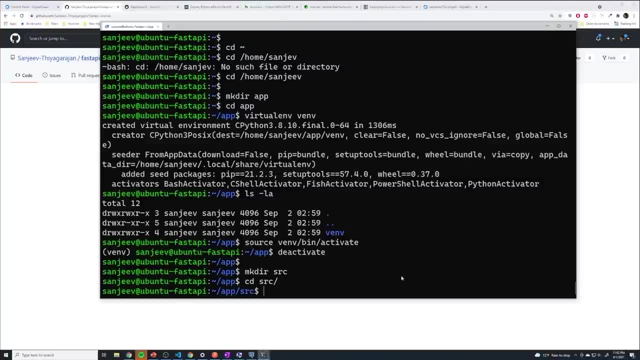 And once you get to the repository, this is going to be the URL. Or you can just select code right here And then this is going to give you a little link to copy. So we can just copy that. And then we can go back here and we can say: get clone paste that in here. 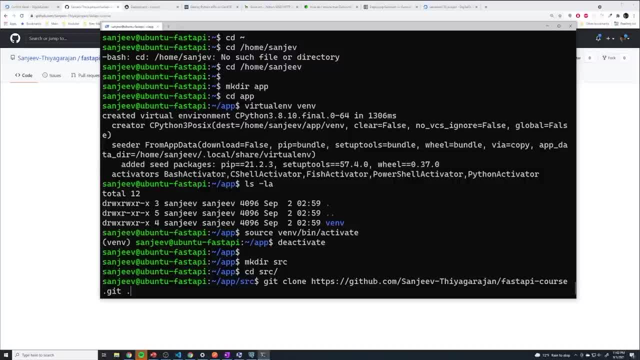 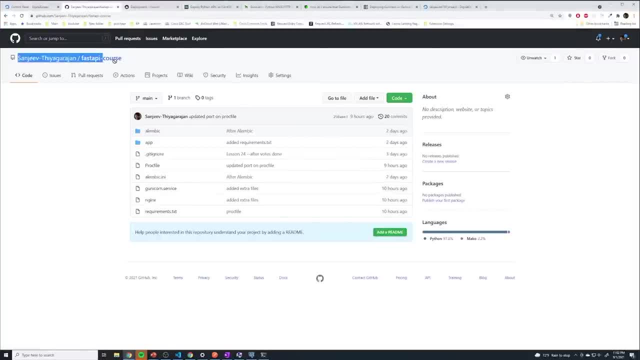 And then before you hit enter, hit space And then dot. so that's going to install it in this current directory and it's not going to create another directory. That's the name of my repository, which is kind of annoying. I don't actually want a directory called fast API, dot course. 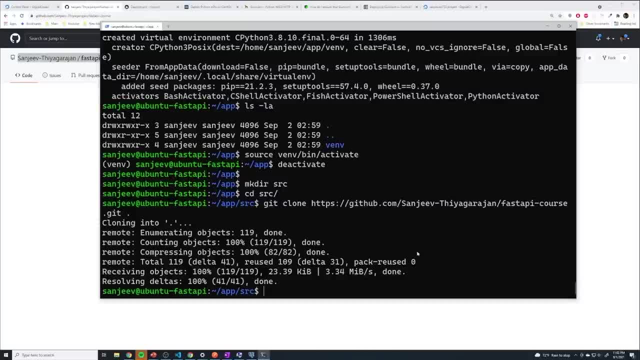 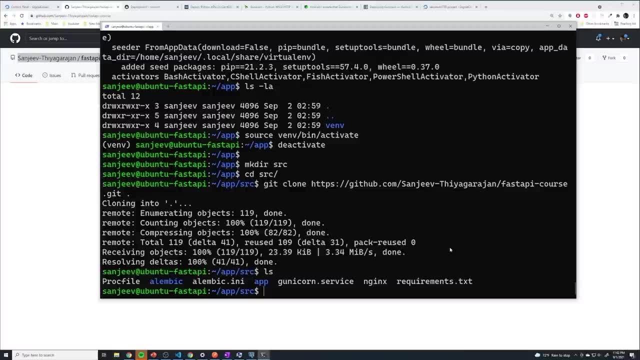 So we'll hit that, We'll run it. It's going to clone it And at this point, if I do an LS, we should see all of our specific code. Great. Now, before we do anything else, let's reactivate our virtual environment. 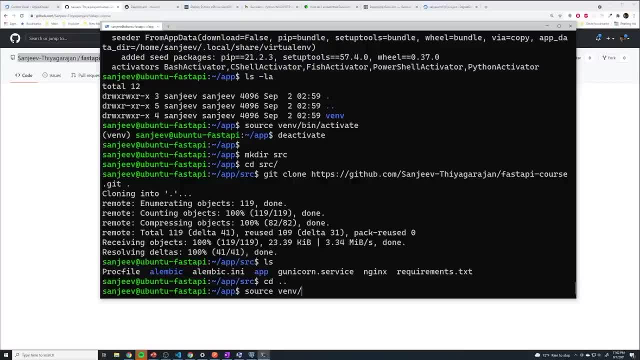 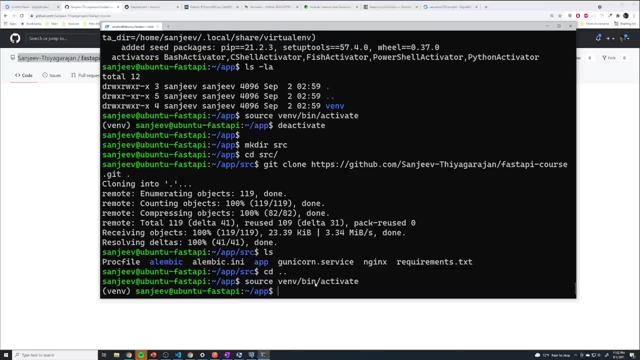 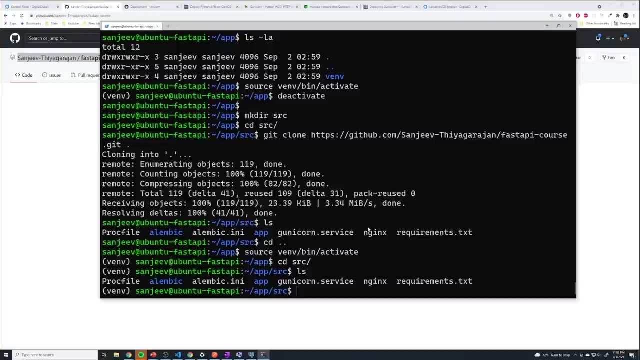 So we'll say source vnv lib- sorry, not lib- bin activate. right, we've got our virtual environment set up again And we're going to move into our source directory. And if you recall, remember we don't have any packages installed. 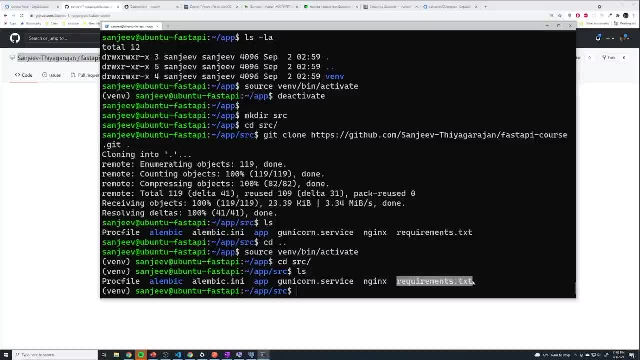 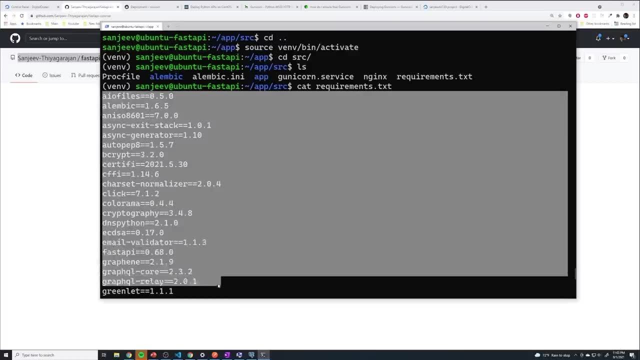 So we don't even have fast API installed, But we do have our requirements dot txt file. So if I just cat that real quick, if you forgot what that was, that's going to tell this machine exactly what version of every single file. 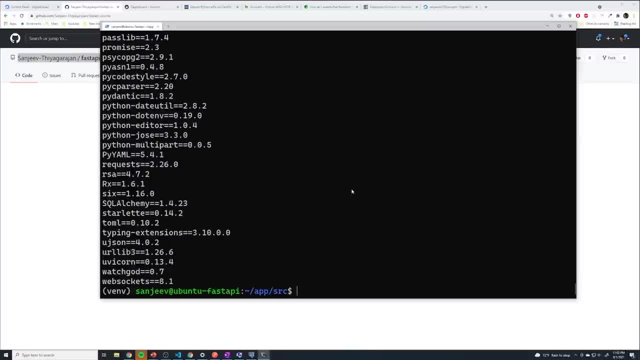 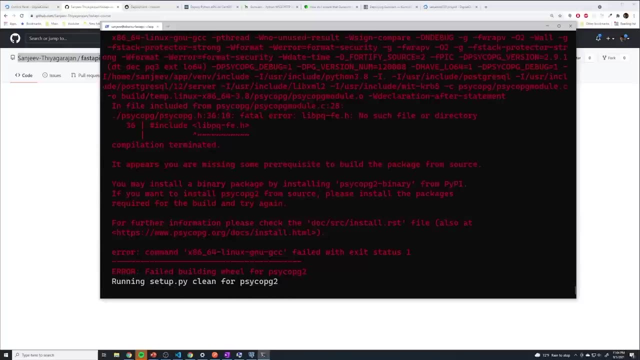 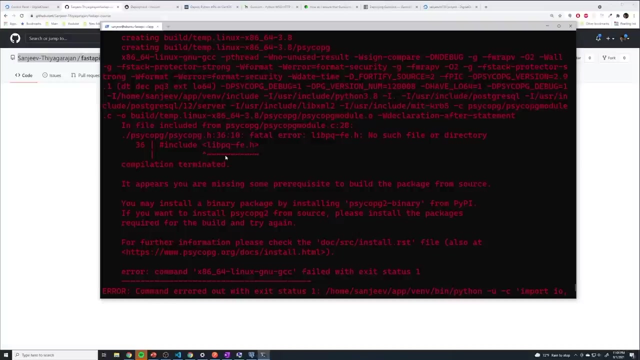 Dependency we need to install for our application to work, And so we can just install all of those with one command by doing pip. install dash our requirements dot txt. All right, so I got an error, And this was expected on my end, because when I was running through this, I ran into this. 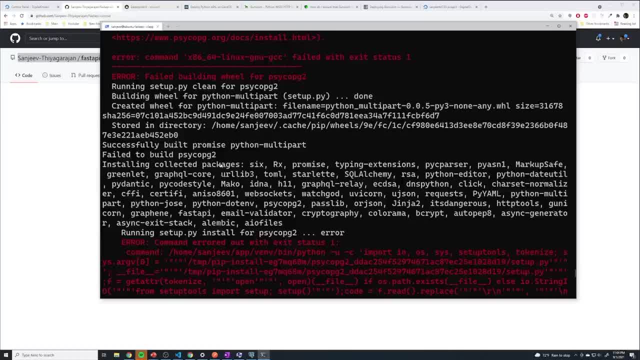 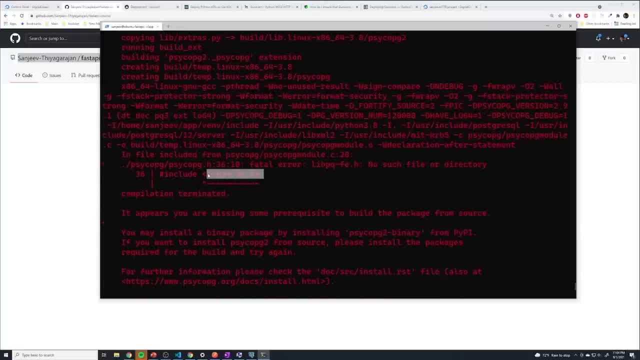 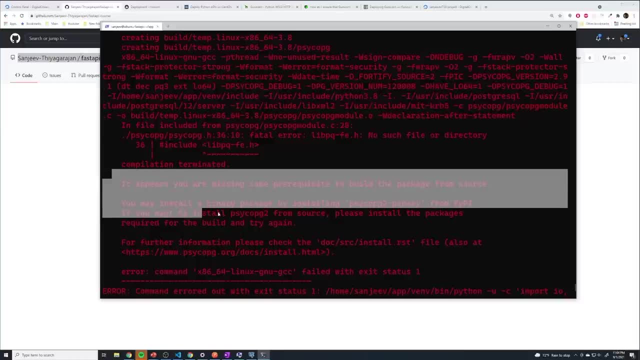 then lib pq, dash fv dot h. This is implying that we're missing a package that's probably called lib pq. If you actually search this error, you're going to get the same result. So if you run into this exact issue or even another issue, just look for the library mentioned. 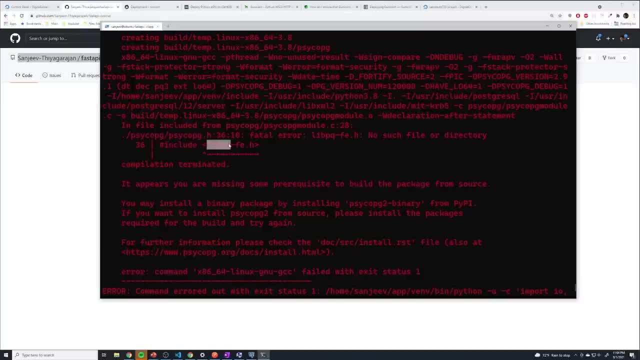 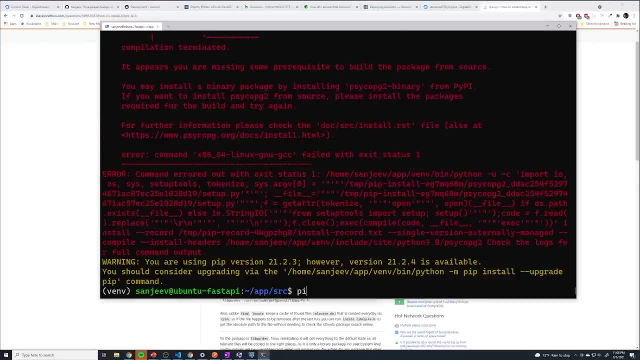 right here where it says that include line right and just search for that library and just see how to install it. Okay, so it's. since it said we're missing this library, I'm going to do a- sorry, it's not actually a pip install. 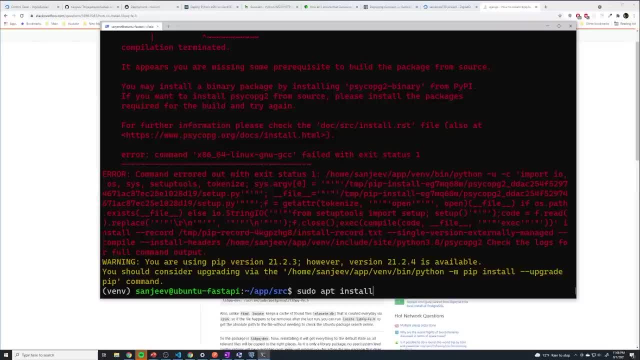 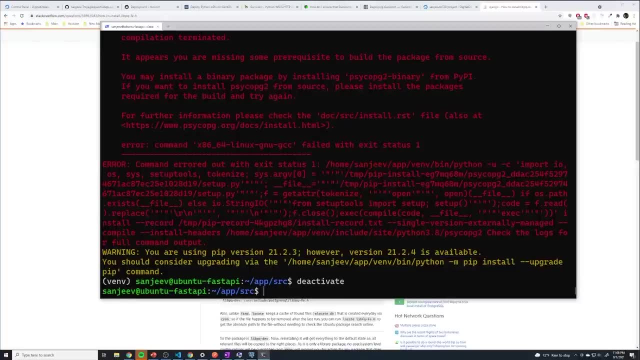 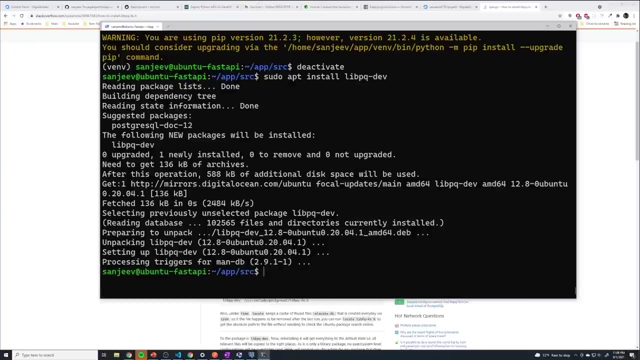 We have to do an apt install. So we do sudo apt install And actually, before I even do that, I'm going to deactivate my virtual environment And we're going to do a sudo apt install. lib p q dash dev. Alright, so now that we've got that library, that missing library, installed, 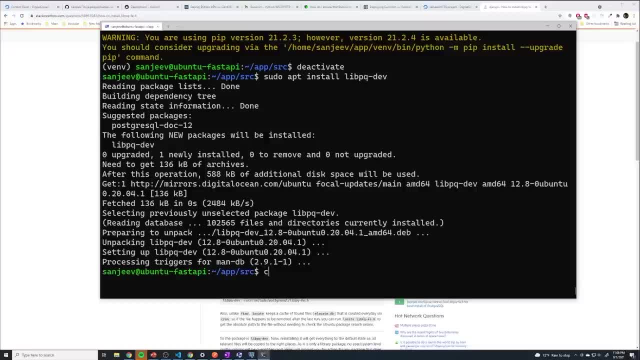 we're going to then go back into our library. Okay, so now that we've got that missing library installed, we're going to then go back into our virtual environment And we're going to run that same command to install all of our requirements. 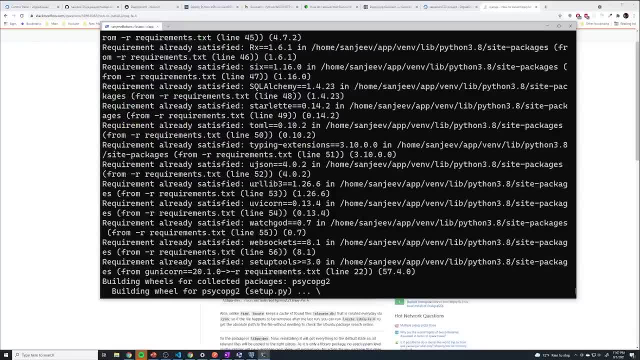 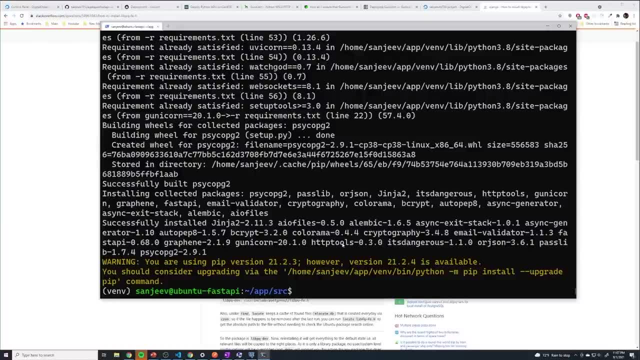 And I have to move into my source folder. Alright, and it looks like we have successfully installed all of our packages. The next thing that I actually want to do is: let's go ahead and try to start our application. So let's go ahead and try to start our application. 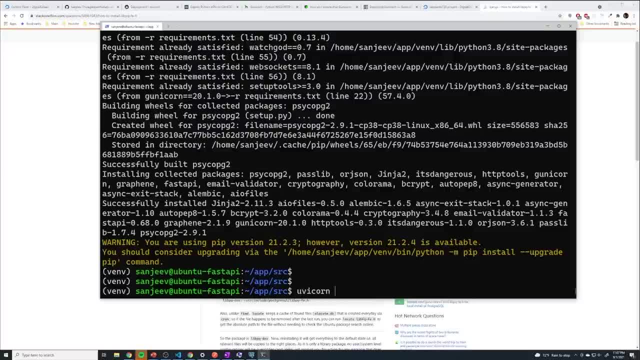 So we have access to UV corn so we can just do a UV corn app dot main. So this is the same exact command that we ran on our local machine and then app. We don't need to pass in the reload flag because this is our production server. 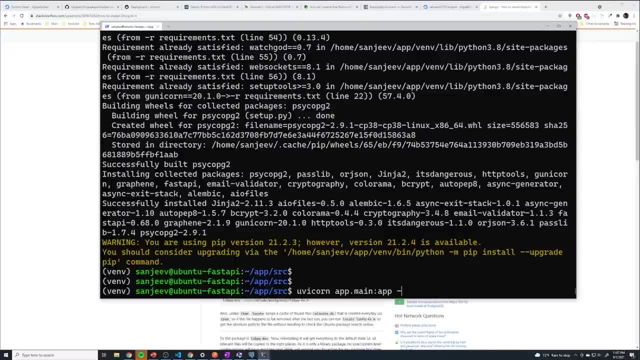 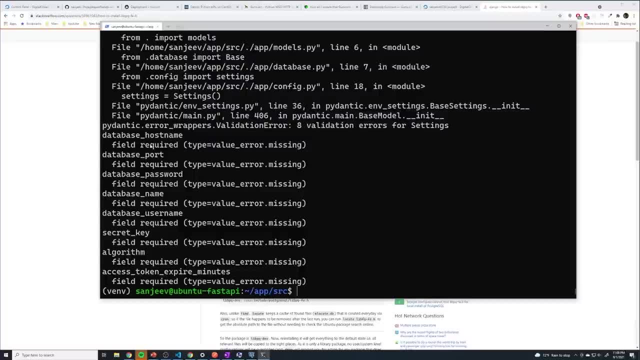 So we would never want it to automatically reload on changes, because no one should be making changes on our production server. So we'll run this and let's see what happens, And it looks like we get eight validation errors, which is to be expected because it. 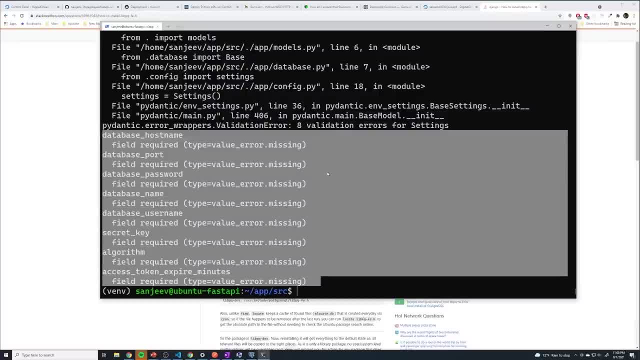 looks like we are missing all of our environment variables, And that's correct. We never set our environment variable. So in the next section, we're going to take a look at how we can set up our environment variables on our Linux machine. Okay, so let's get started on creating our environment variables. 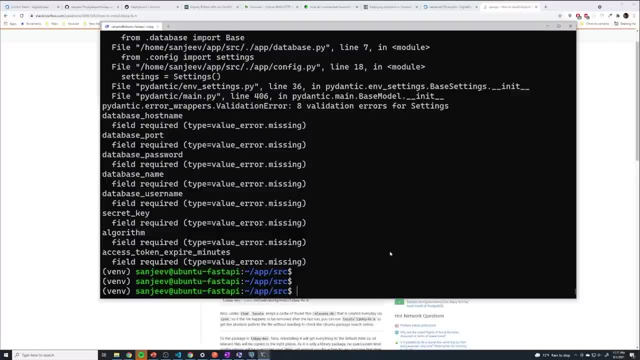 So what we want to do is to create an environment variable on a Linux machine. we say export And then we give the name of the variable. here This is just a demonstration, So I'm going to say my underscore name And then we set equals and then whatever value we want to give it. 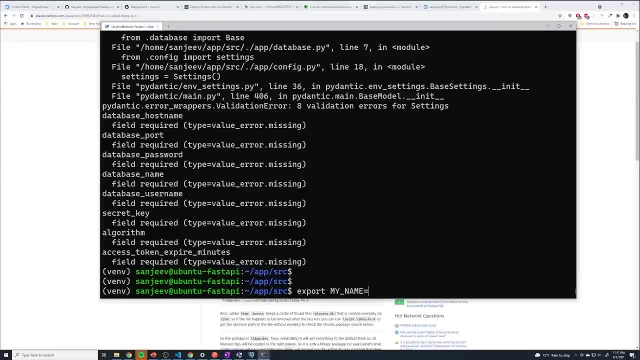 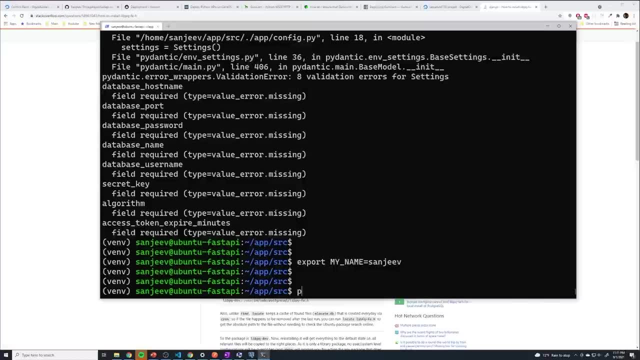 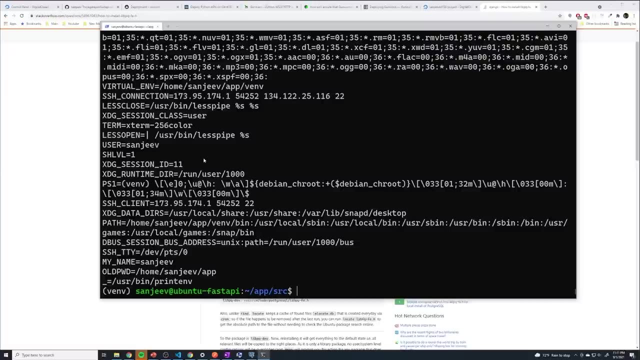 So you can give it anything. This is Angie, alright, so we'll hit that, we'll run that And then to actually see if this worked, to see all of your environment variables, we just say print and V, And so this is going to spit out a whole bunch of default environment. 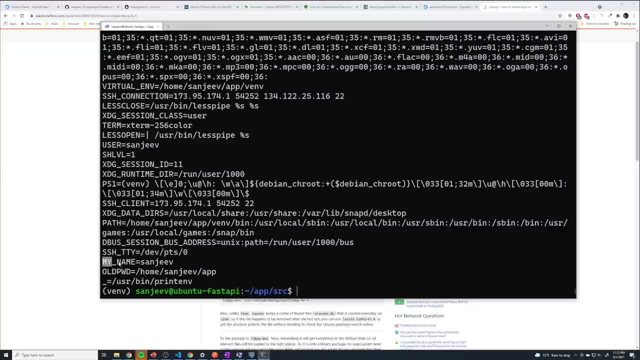 variables And then to see the one we sent, just kind of look down, look for my name, and we can see that it was successfully set. So at this point we can just go one by one and manually set all of these. However, that is a very inconvenient process. 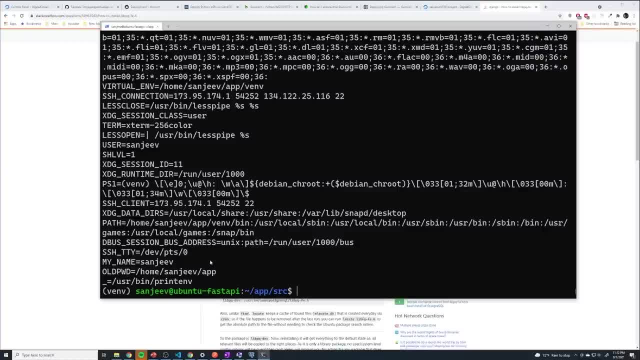 And I wouldn't expect you guys to do that, Because you know we've got seven or eight and any other project could have 10 2030.. So it's not really realistic to do that. you know one environment variable at a time. 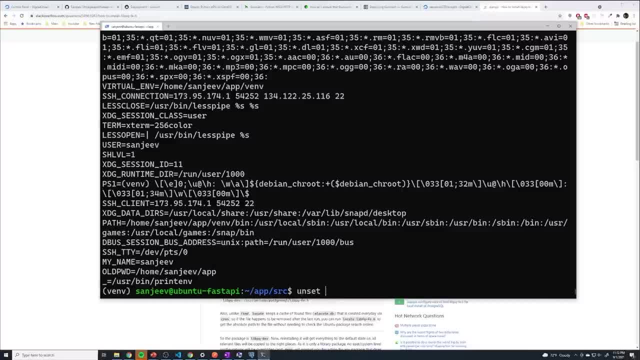 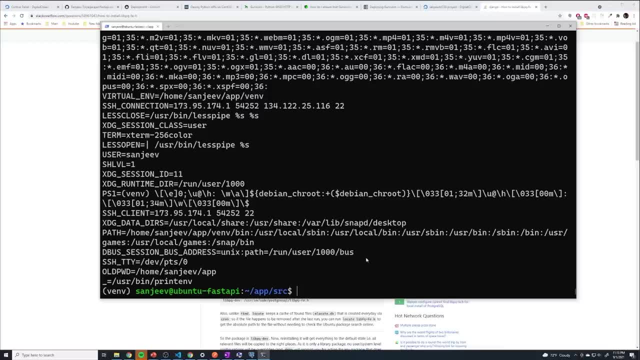 So let me quickly remove this environment variable, which you can do with the onset command, And so I could just say unset my underscore name And if I do a print and V, we should see that it's no longer there. And what we're going to do is I'm going to go back to my home directory because I don't. 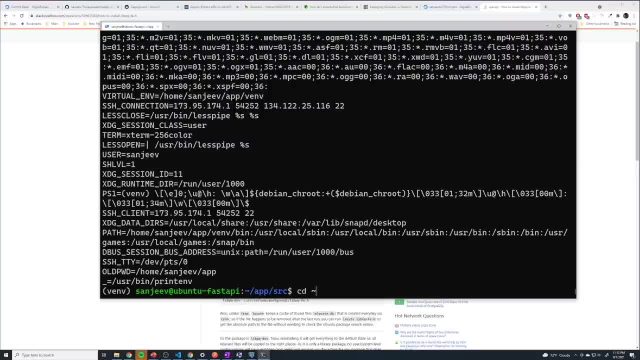 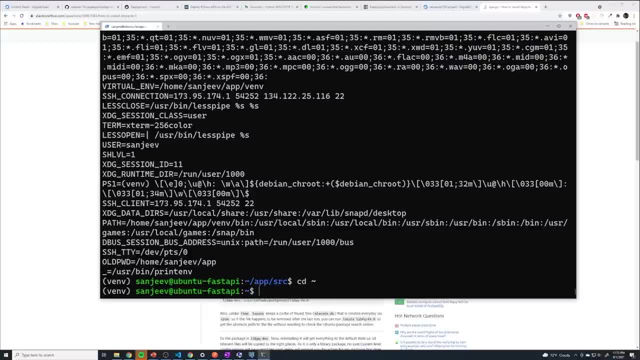 want to mess around in my application directory. I'm going to go to CD and then the tilde, or you can do slash home, slash and then whatever your username is going to do that, right? so this is going to take me back to my home. 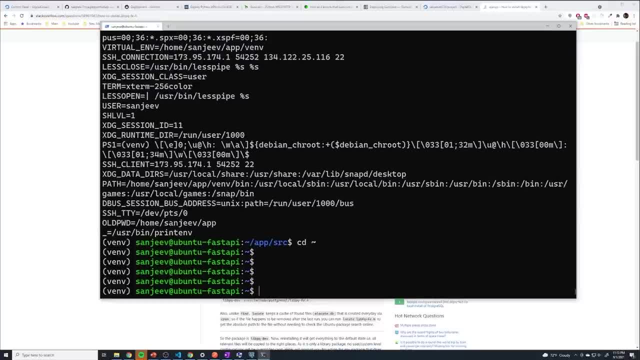 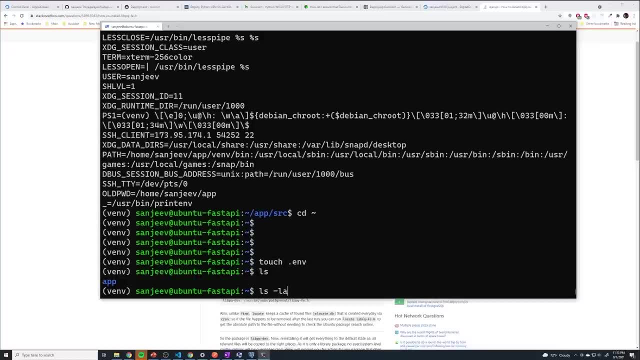 directory And I'm going to create a brand new file. And if you want to create an empty file, you can just say touch, and then I'm going to just call this Env, Alright. so we shouldn't do an LS minus la, we should have theenv file right here. 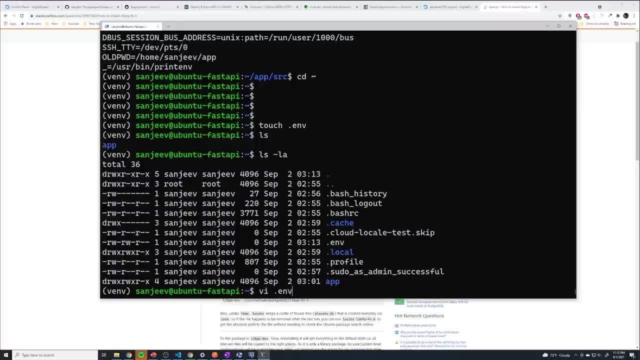 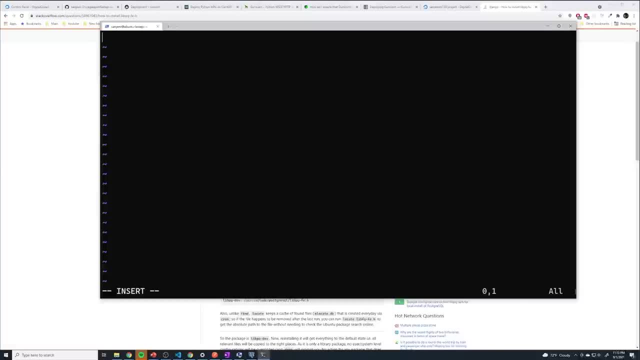 And I'm going to open that up And here I can provide a list of all of the environment variables. So I can say and keep in mind, this has to be in the same exact syntax. So we have to say, just like we would put on the CLI, we'd say export, then the name of 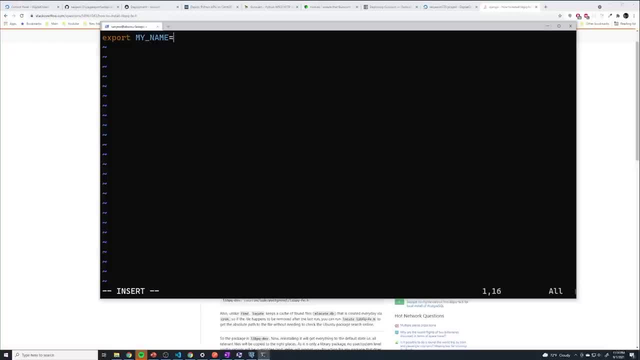 the variable. So I'll say: you know my name again, Chico Sanjeev, And then let's, maybe let's do my underscore password, which is going to be password 123.. So I can save this file And I'm going to go back here. 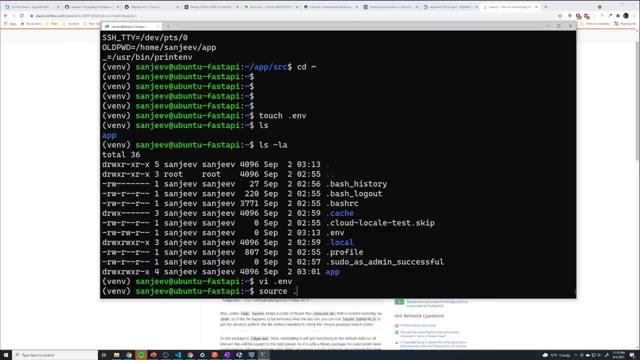 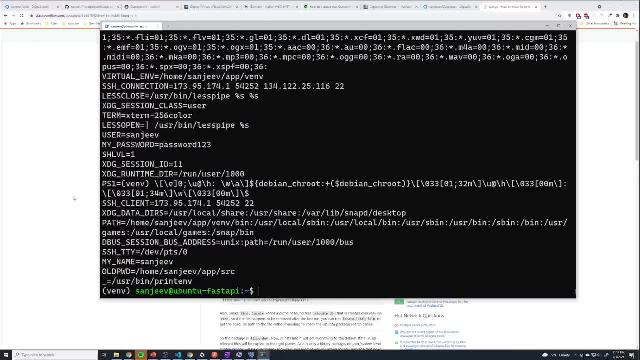 Okay, And I can say sourceenv. So this is going to set all of those environment variables. So if I do a print n v now, we do have my name And somewhere along here we've got my password. So that's another way of setting things. 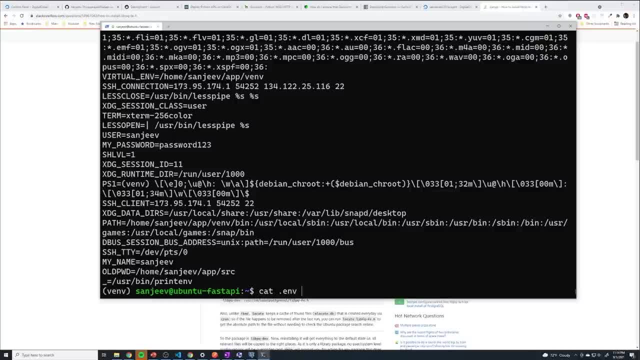 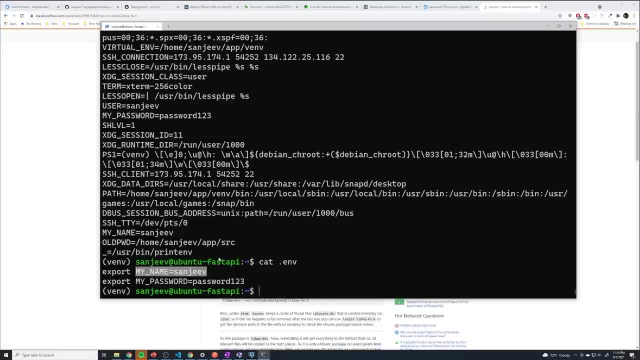 It's a. it's a little bit easier to kind of keep everything in a file, But what I don't like is that I have to put it in this format where I put export and then the environment variable. What would be awesome is if I could just somehow. 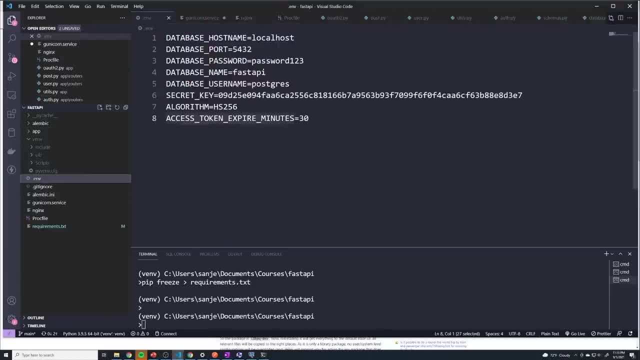 Get it so that the environment variable file in my Ubuntu machine matches with the environment variable file on my local machine. I want to just be able to put the, the key and the value pair like here, And so that way I could just copy this, paste it into my production server and just change. 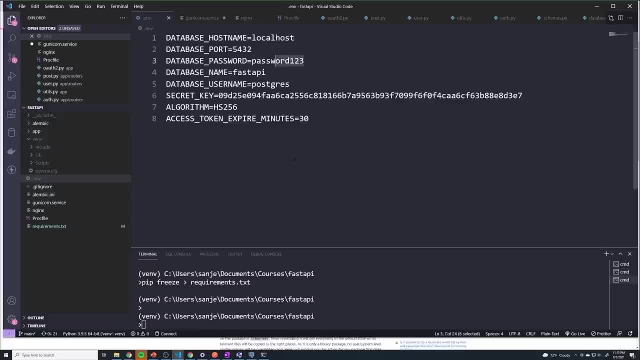 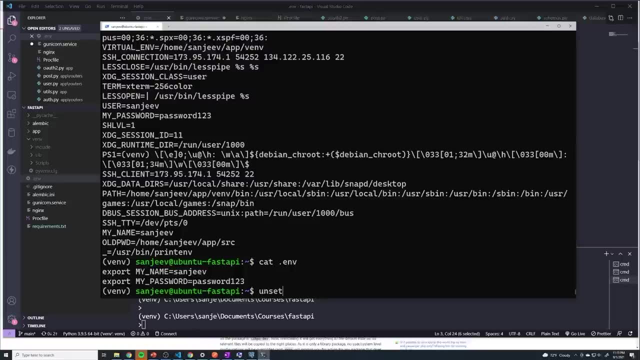 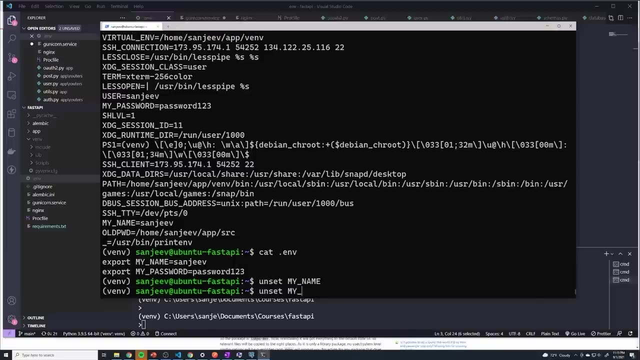 the values there, And so we can actually do that. it just requires a little bit of a modification. So let's go back here And I'm just going to unset both of these real quick And we'll just double check. it got removed, so they're removed. 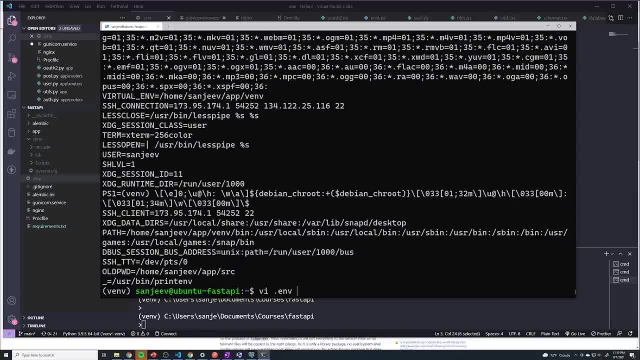 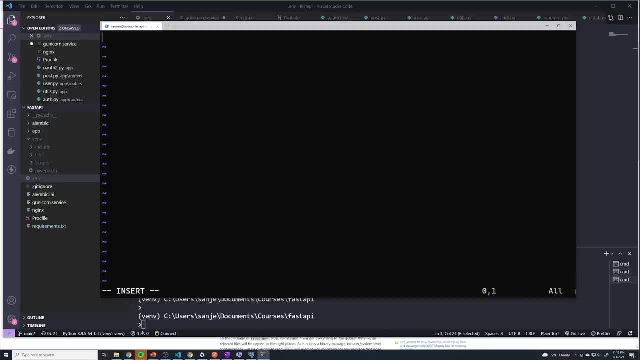 And we're going to open up the dot env file And I'm going to just delete everything, And what I'm going to do is I'm actually just going to copy this for now and just paste it in there. Let's just see if I can get all of this set from a file. 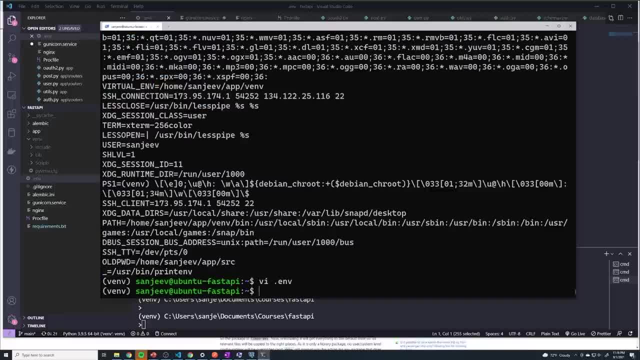 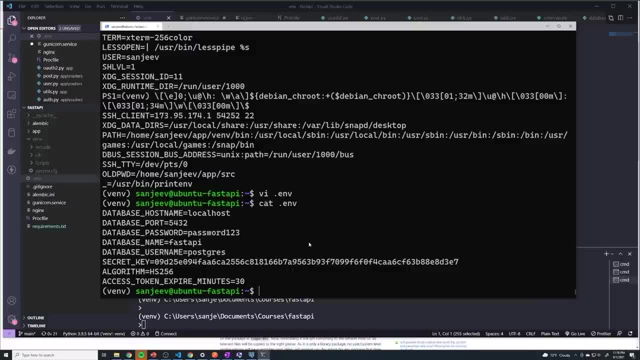 And then we'll change it, And then we're going to paste those values later. And so when you have a regular file, like the one we have right here, where we don't have the word export in front of it, it does require a little bit more of a complex command. 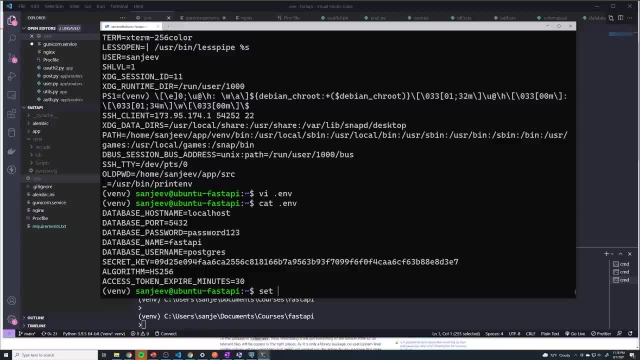 But all you have to do is you run this command So you do set dash o all export, then source, And then you provide the path to the file. So this is going to be my home directory, So it's slash home. 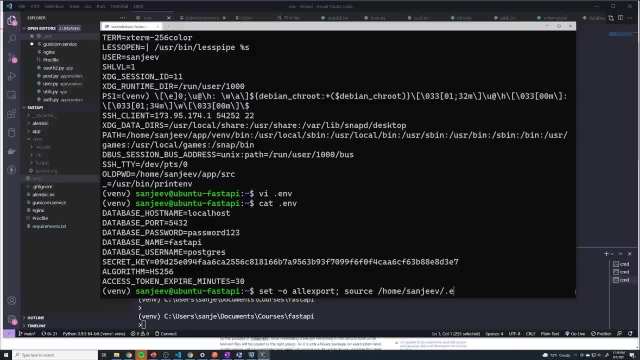 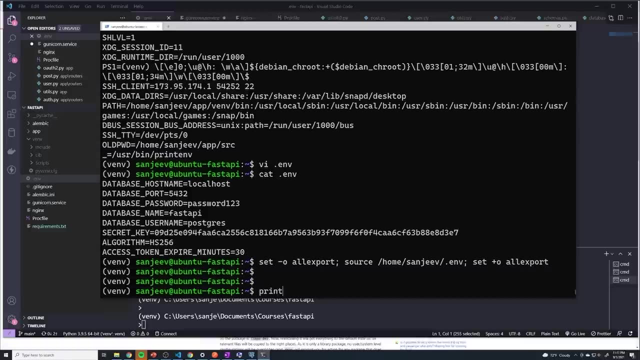 slash Sanjeev, just make sure you swap it out with your specific username. And then we provide dot env And then we say: set plus. oh, all export, All right. And so now, if I do a print nv, we can see: I've got my database password, my database. 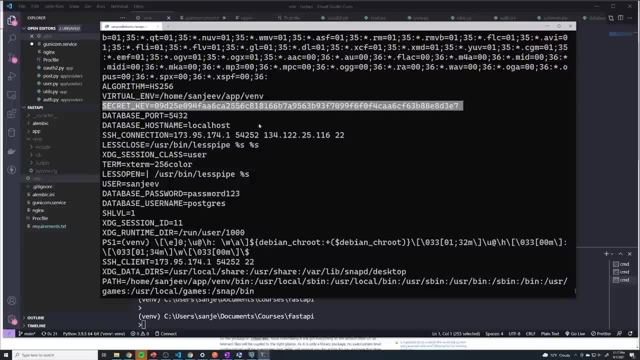 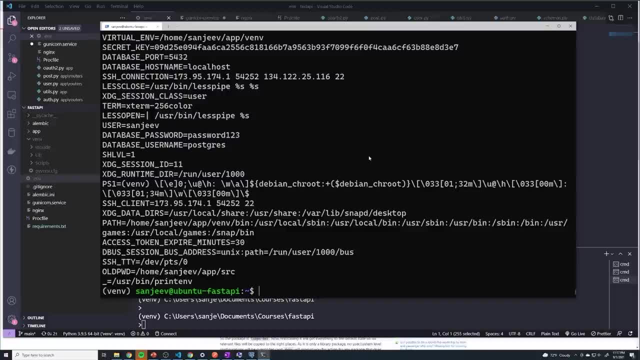 username, I've got my database, port, hostname and all of the variables that I set have now been set as environments. So that's what we're going to do. However, there's still one minor issue: If I exit out of here- or actually, sorry, not if I exit- if I reboot. 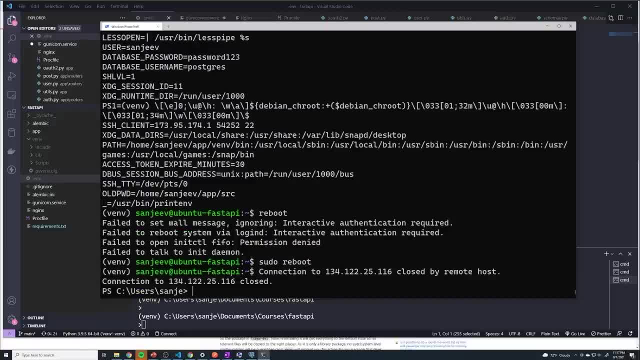 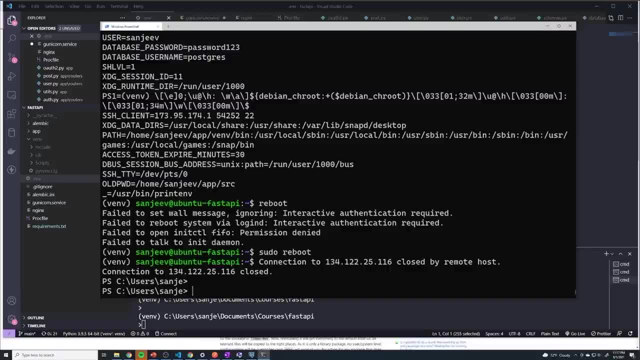 And I actually have to do a pseudo to actually reboot. but I'm going to reboot and I'm going to show you guys that when you reload your machine you lose your environment variables. So we'll give this about a minute or two to kind of boot back up. 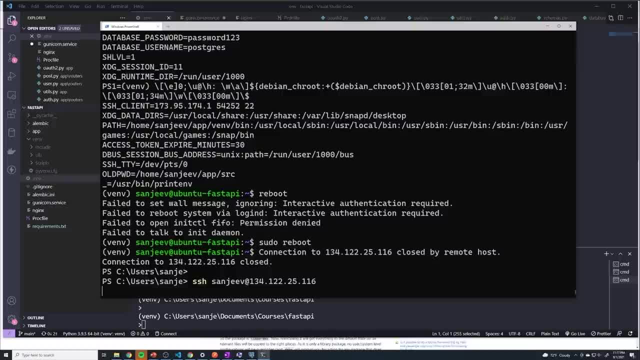 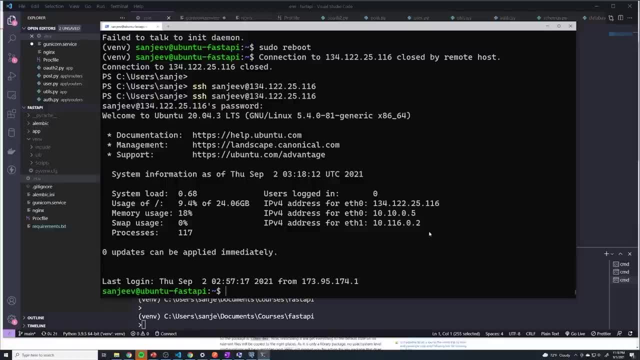 Although I find a bunch of machines boot up fairly quickly. So let's just give this a shot, See if we can connect. No, not yet All right, so I've logged back in after it rebooted. If I do a print nv, you're going to see that all of the environment variables that I set. 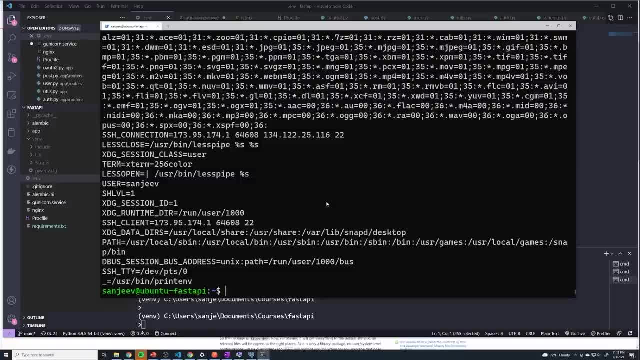 are all now gone. So how can we get all of these environment variables to persist? through a reboot, Because if our machine goes down, comes back up, then we lose those environment variables, then our application is broken. Well, there's a couple of different ways that we can have environment variables persist. 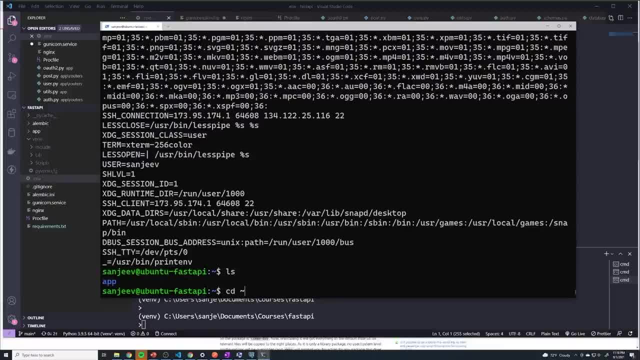 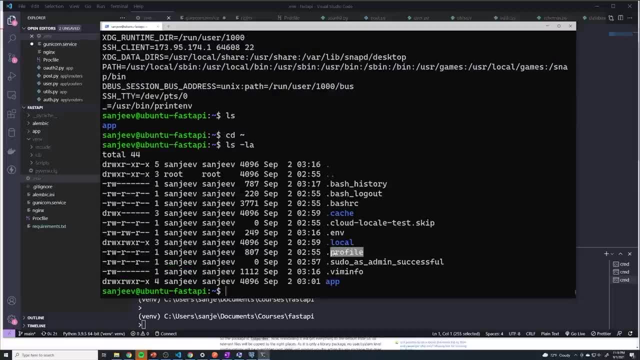 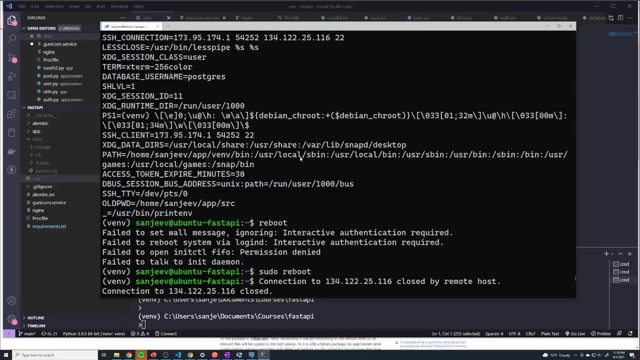 Through a reboot. One of the ways is: let's go to our home directory. we're going to do an ls minus l a, And what I'm going to do is we're going to go into this dot profile file And we're going to set that exact command that we had run to set my environment variables. 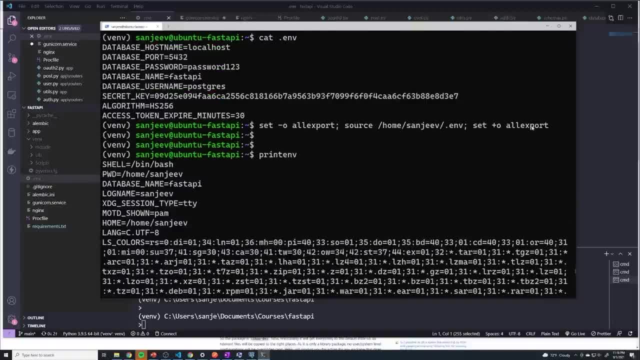 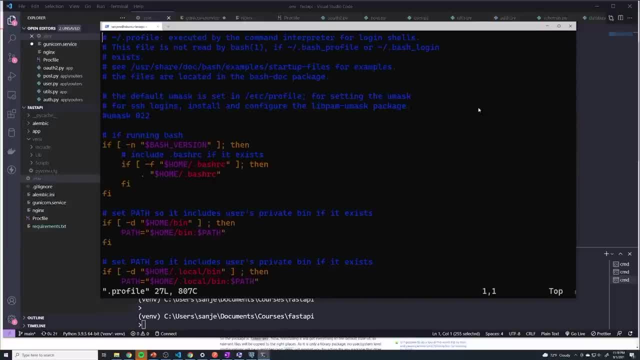 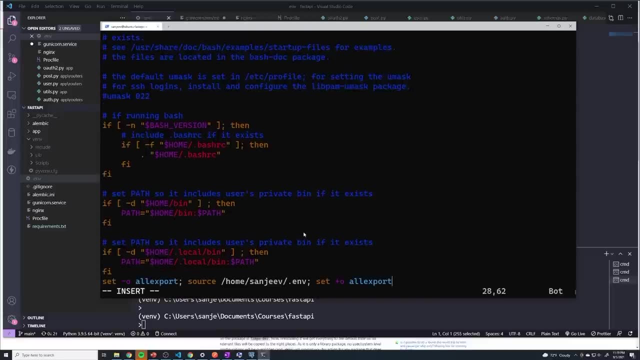 Where is that command, this one, right here in that file. so copy this And then just do a vi dot profile, Okay, And then go to the bottom of the file And below the last line just paste that command in, And then we can just wq. 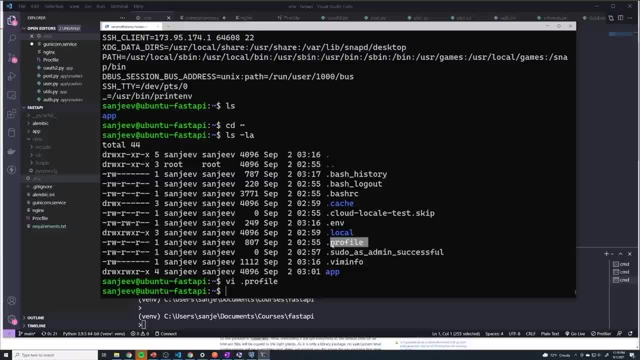 Alright, and so this is going to cause: anytime we open up a session or a terminal, even through a reboot, it's going to run that specific command so that those environment variables are all set. Right now, if you do a print nv, you will see that it's not set. 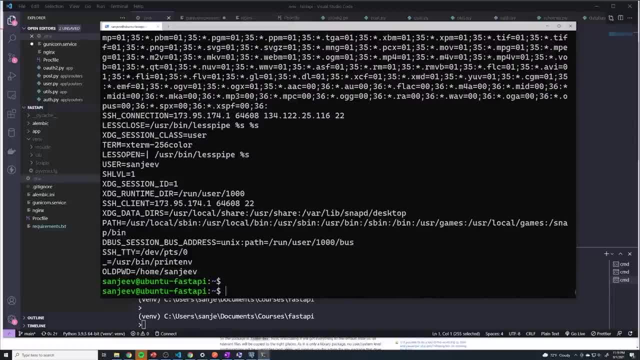 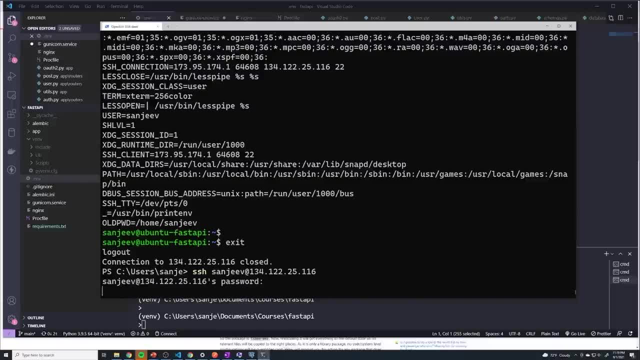 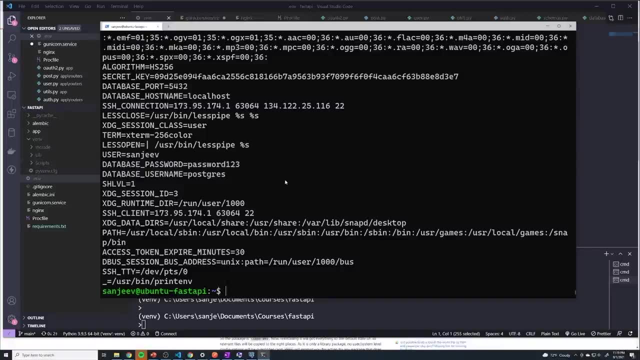 And that's to be expected Because we were already connected To it. but if I exit out of here, reconnect, do a print nv. we can now see that the our environment variables are set And then, just to prove to you that this actually persists, through reboot. we're going to reboot. 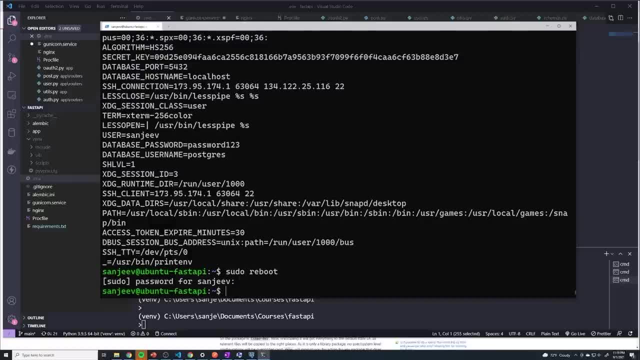 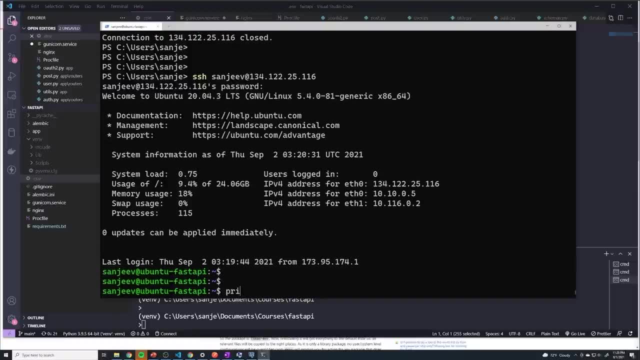 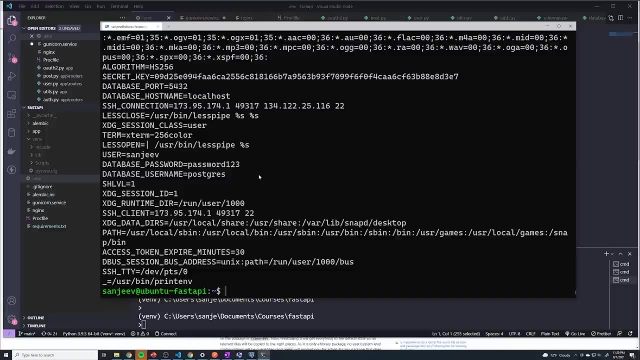 this machine Alright, so it's rebooted. Let's do a print nv, And, And we can see all of our environment variables are still set. So this is the method that I'm going to go with. Keep in mind, when it comes to environment variables, there are 1000 different ways to. 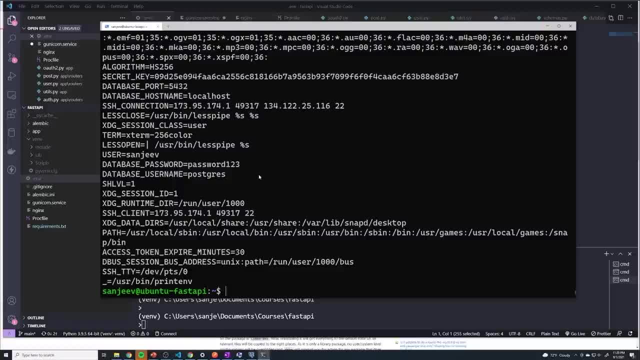 tackle this, And so people like to set their environment variables in different ways. This is just the way that I've done it. This is the simplest way, But there are, you know, a number of different other methods. some of them will probably 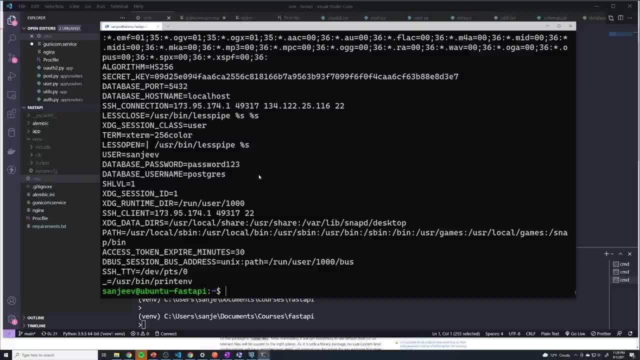 be more recommended better, But I want to keep things as simple as possible. The one thing I do want to kind of highlight is that our environment variables are set. This is just the way that I've done it. This is the simplest way. 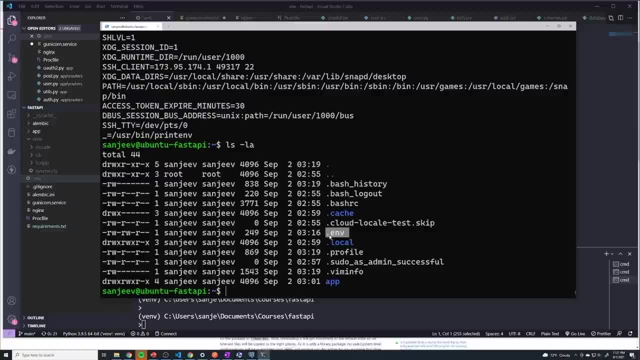 But there are, you know, a number of different other methods. Our environment variable is stored in my home directory. It is not in the app directory, where all of my application code is, And that's important to me, because I don't want to put it in my application code. 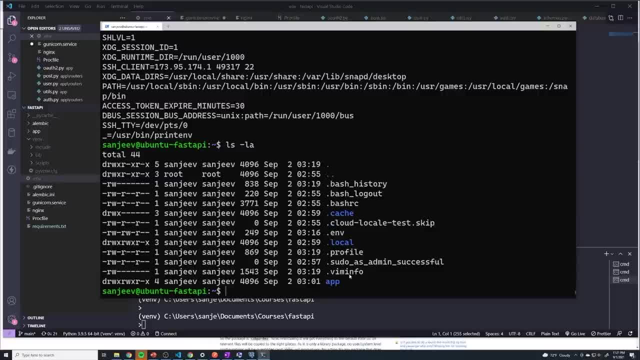 Because I don't want it to accidentally get checked into git. I don't want anyone to accidentally see my production passwords or anything like that, Because then my entire application is compromised. So I like to keep it separate by moving it into a completely separate folder so that 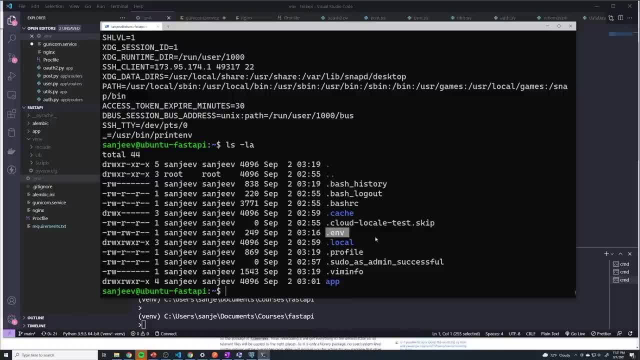 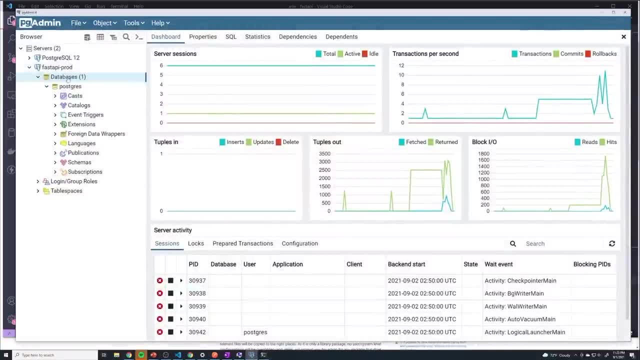 there's no chance that it gets mixed up in my application code. All right, so since we can connect to our Postgres database, let's go ahead and actually create the database within this machine. So I'm going to select right click here and I'm going to say: create database, call your. 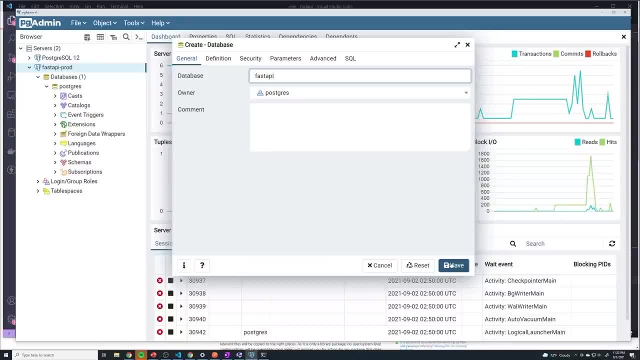 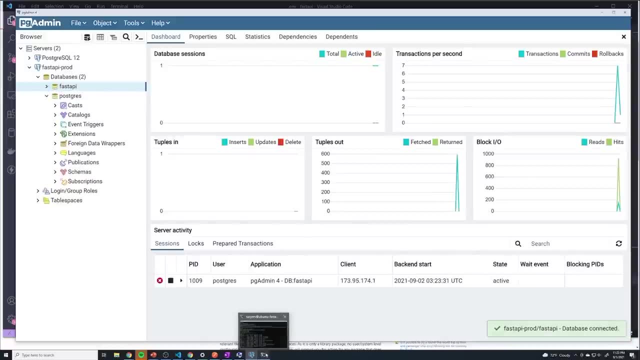 database or whatever you want. I'm just going to call it fast API to keep things simple. And so now we have our database once we click on it, And so now it's up and running. And so, since we have that information and we have the information for connecting to 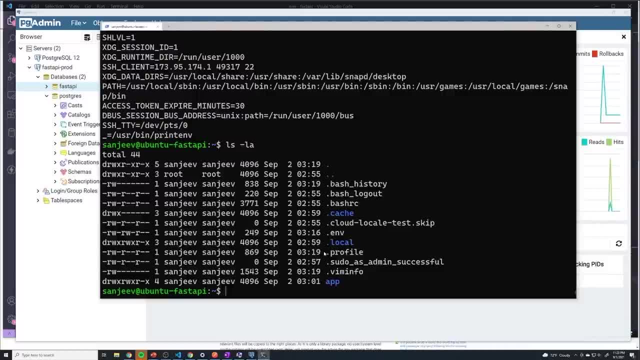 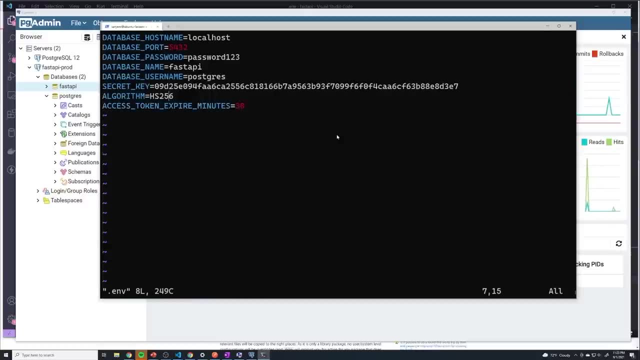 our actual Postgres instance on this machine. let's update these environment variable files so that they are accurate at this point, Because I believe they're still pointing to whatever our production was set as- Sorry, our development environment. So here the host name is still going to be localhost. 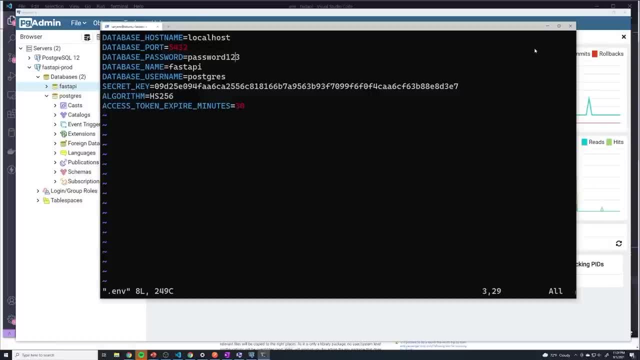 The port. since I installed Postgres on the default port, we can keep that the same. You want to make sure you update your production password? I chose the same exact password, just to keep things simple. The database name: we just created, one called fast API. 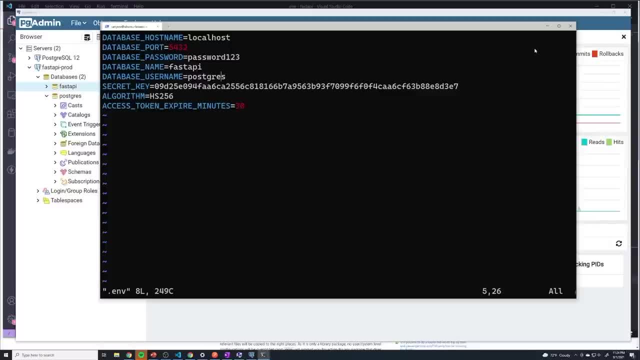 Here The database username. if you want to, it is recommended to create another Postgres user. However, I'm just going to keep this as the default Postgres user, to keep things as simple. You definitely want to upgrade, update the secret key, the algorithm. you can leave that. 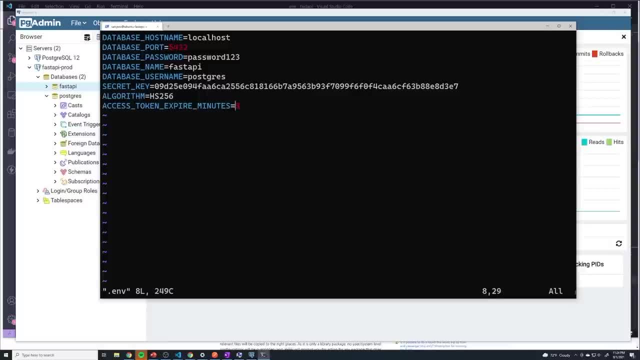 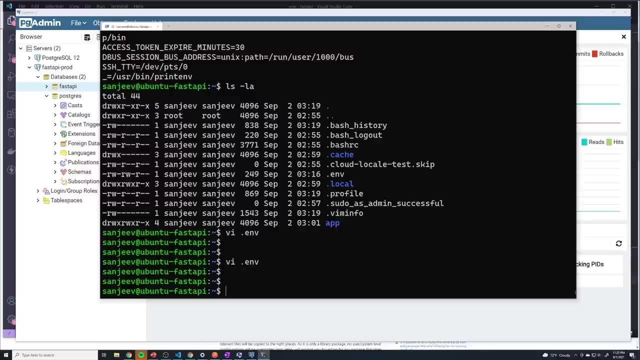 as default, And then the access token. I'm going to make this a little bit longer. Let's do 300 minutes, All right, And now let's reactivate our environment. So I'm going to go into apps And then we'll do. 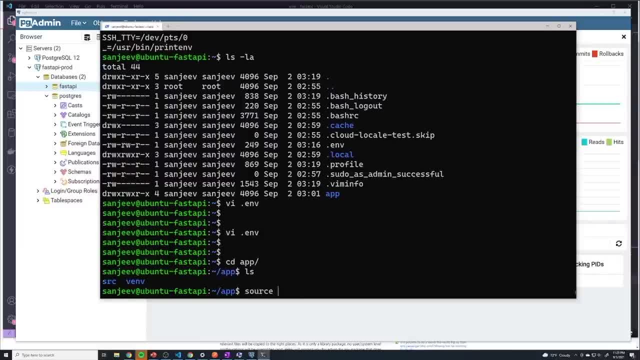 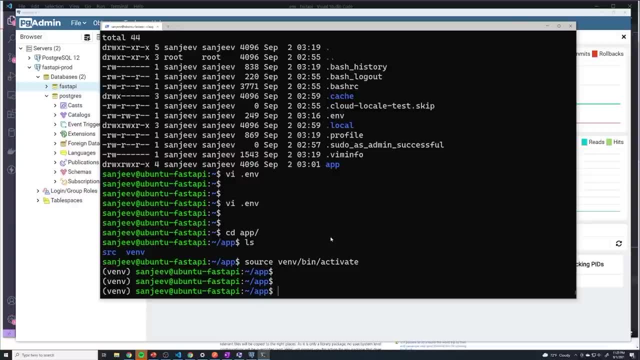 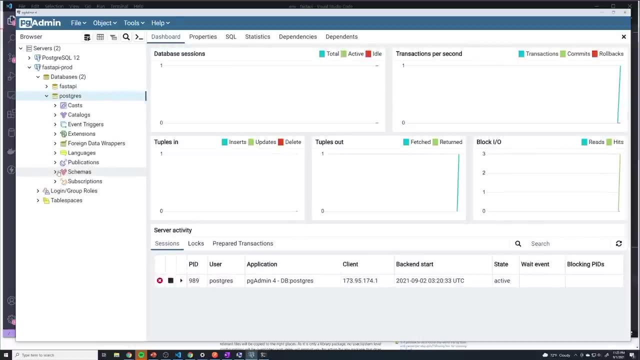 source, the envy been activate. that's going to activate our virtual environment And right now you probably notice a little bit of an issue And that is that we don't have any tables. right now You go to our schemas And then our. we got no tables in here. 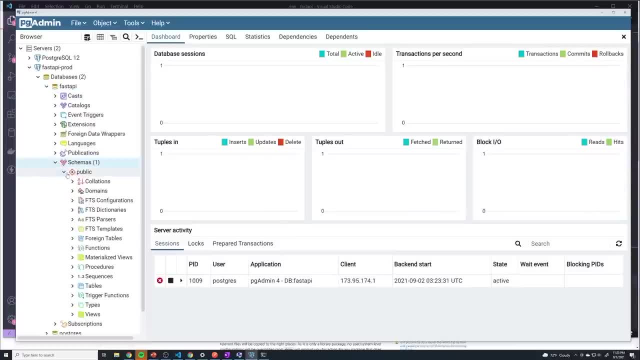 Oh sorry, we're in the wrong database. in the fast API We've got no tables Right, nothing here, And so we have to set up all of our models now. However, since we are in our production environment and since we've set up Alembic, you'll see. 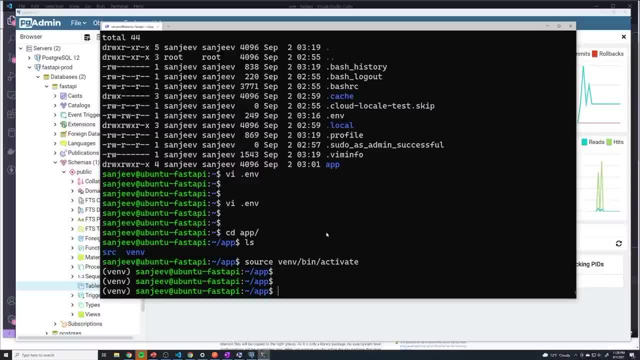 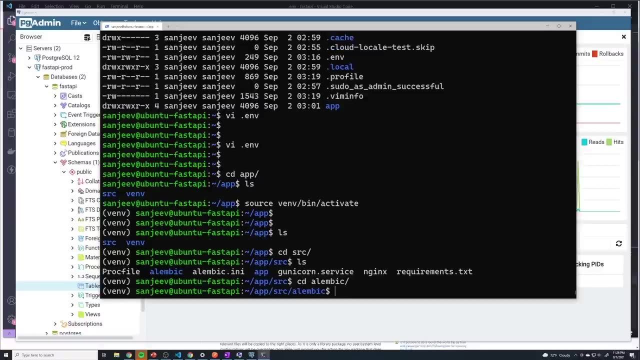 that this is dead simple. And when it comes to Alembic, it's important that in your production environment you never create revisions. in your production environment you only create it in your development environment and you check it into Git. And since we checked it into Git, if we go to source and then go into our Alembic file, 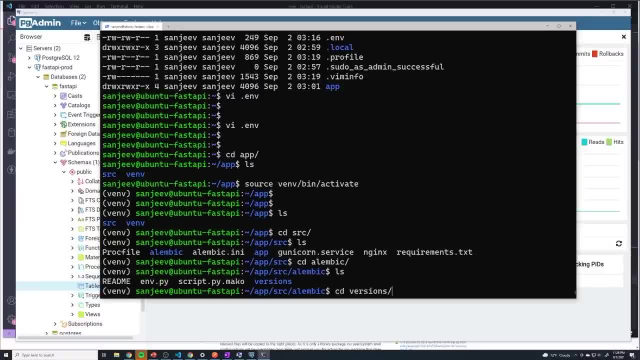 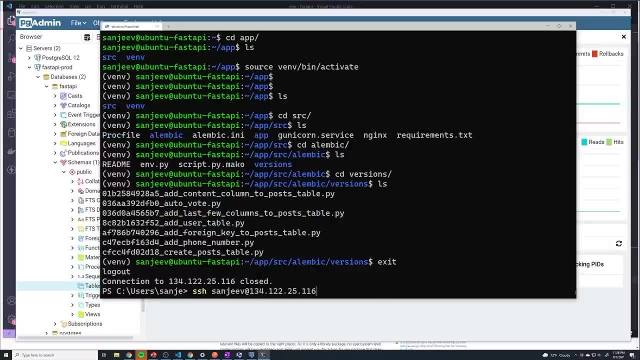 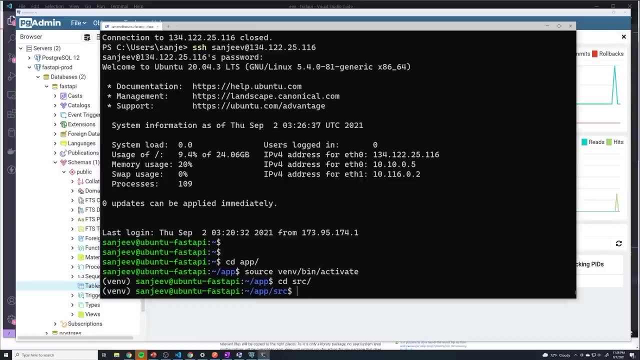 folder and do an LS and then go into versions. we have all of our revision files, And so what we can do is we can just- oh sorry, I didn't mean to hit exit, got logged back in now. All right, make sure that virtual environments enabled every time I'm going to go into source. 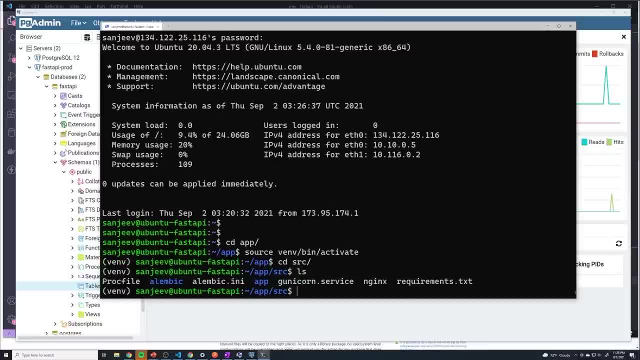 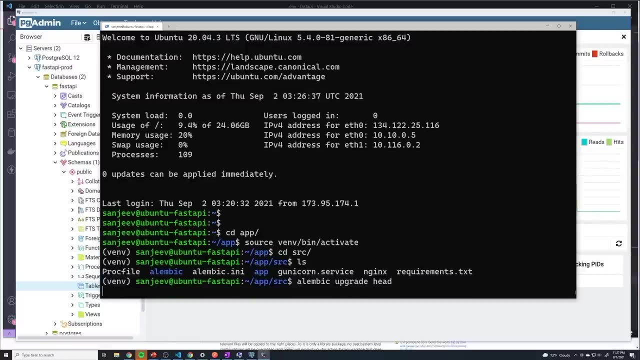 And what I'm going to do is I'm going to do Alembic Upgrade And then head. So this is going to set up our database and it's going to upgrade it to the latest revision. All right, And take a look at that. 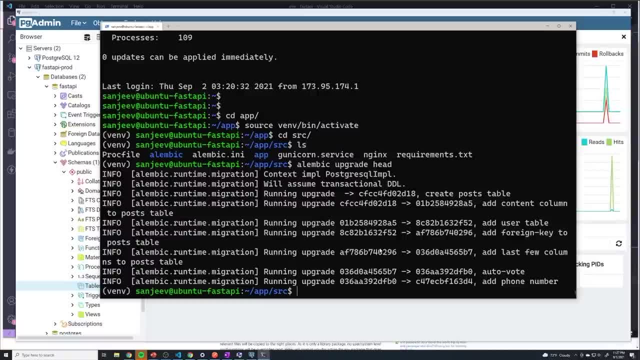 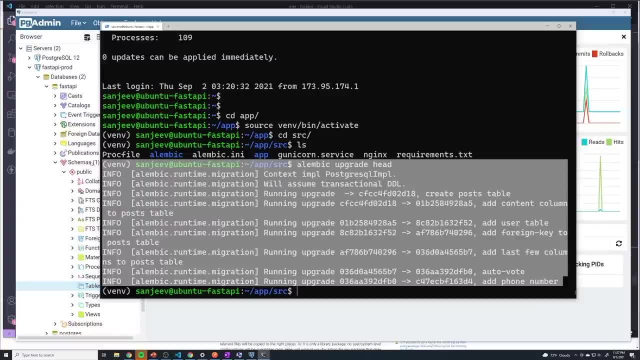 It created all of the individual revisions, one at a time. So we can- we can still roll back just the same exact way that we did in development, And with just a click of a button we've got our entire database schema all set up. 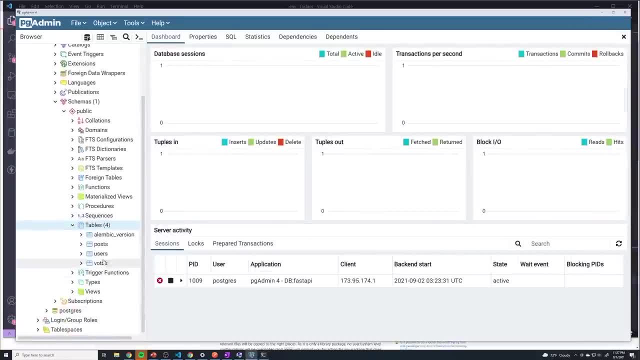 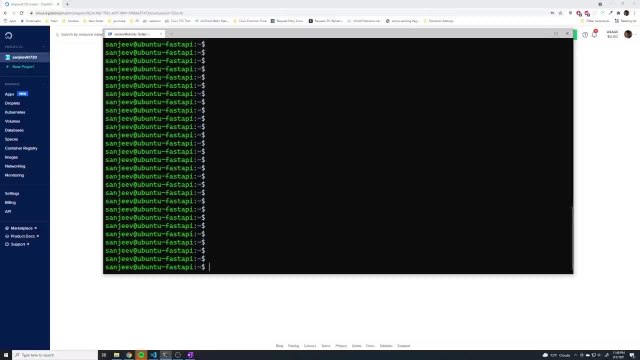 And we can just refresh this real quick And then go into our tables And you can see that we've got our three tables plus the Alembic table as well. So now that we have our database all set, I think it's time we try to start our application. 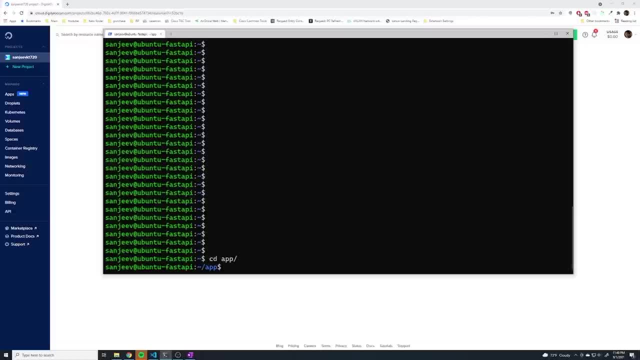 again. So move into your apps directory And if you've already, and if you haven't activated your virtual environment, do that again. Move into the source directory. And now we're going to run the same UV corn command that we ran in our development environment. 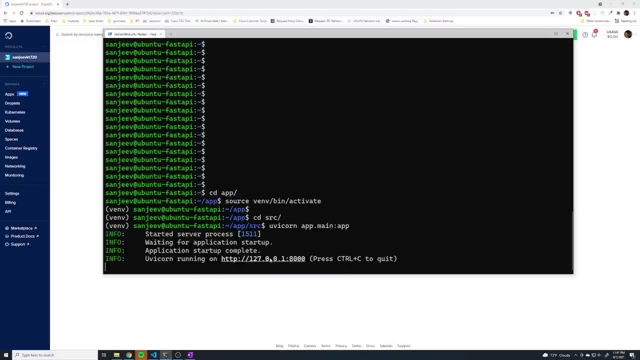 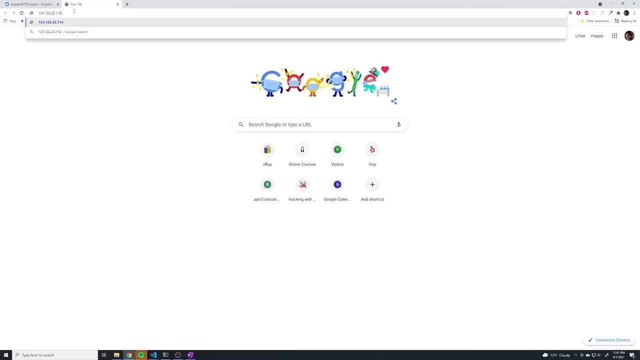 All right. so it says it's running on the local host IP address of this machine on port 8000,, which is the default port, So let's try to connect to it. So what we have to do is grab this And we're just going to paste the IP address into our browser. 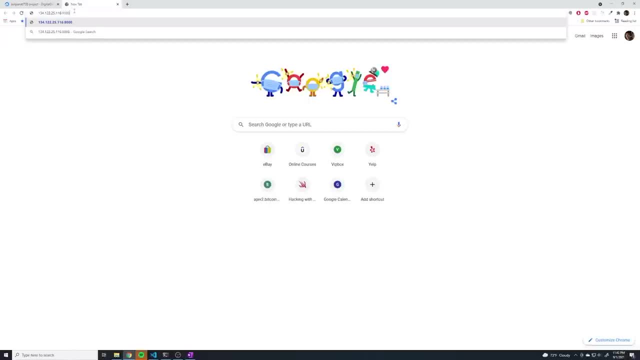 And we're going to do colon port 8000. And let's see if this works. And it looks like it didn't work. So what happened? Well, The problem here is that we needed to make sure that it can listen on any IP address. 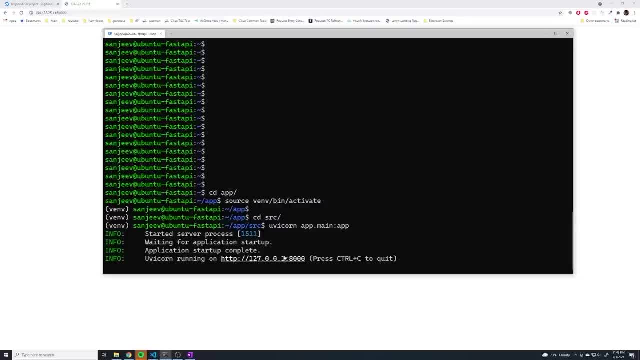 So when you just set this to 127.0.0.1,, that means only this machine can access it. So I'm going to Ctrl C out of this. so we're going to stop it And we're going to pass in one more flag. we're going to say dash, dash, host. 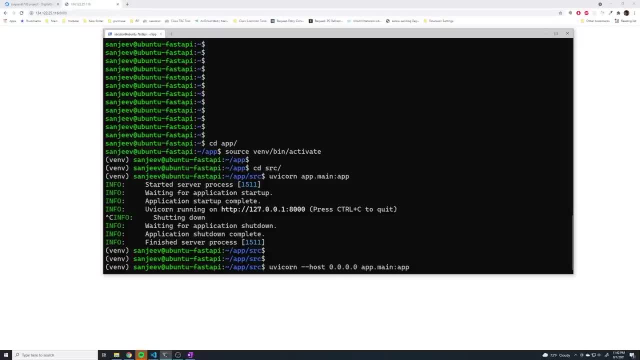 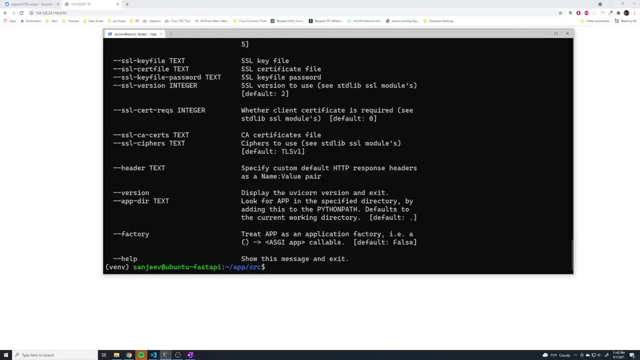 And then provide the IP of 0000.. So we're going to listen on any IP that this machine is potentially running And if you wanted to- if I did a dash dash, help real quick- We can also specify what port we want to listen on. 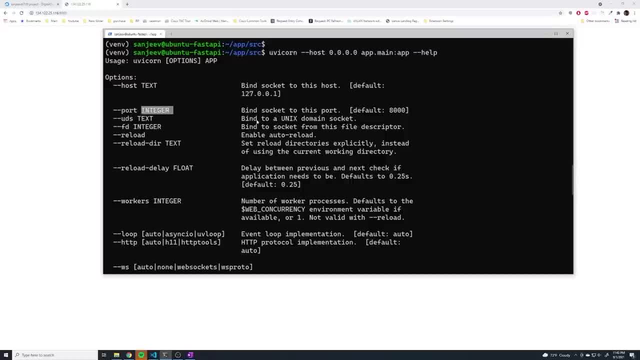 So if I do dash dash port, I can provide a different port so it doesn't go to the default port 8000. But I'm going to keep it as port 8000, you're going to see that it ultimately doesn't matter. 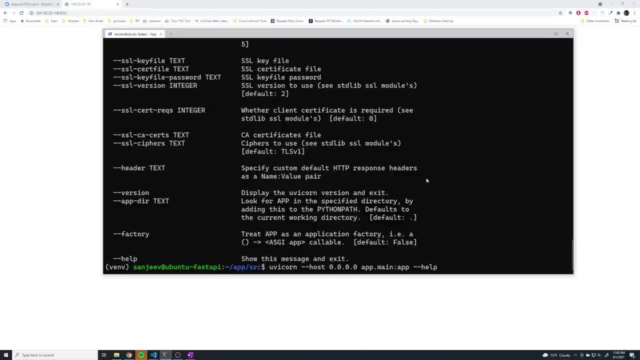 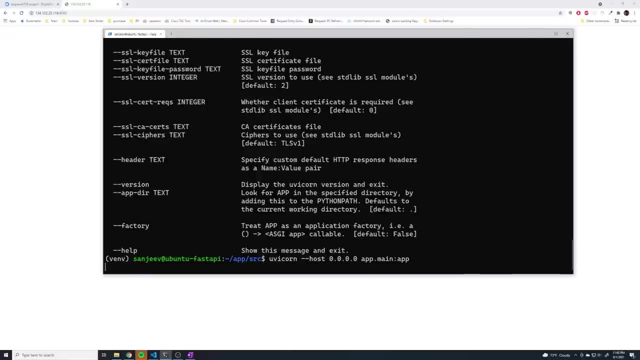 when we actually deploy, because we're going to deploy it in a way that it's always going to use either port 80 or port 443, which is the default port for HTTP and HTTPS. So this is good enough, We're going to start it again. 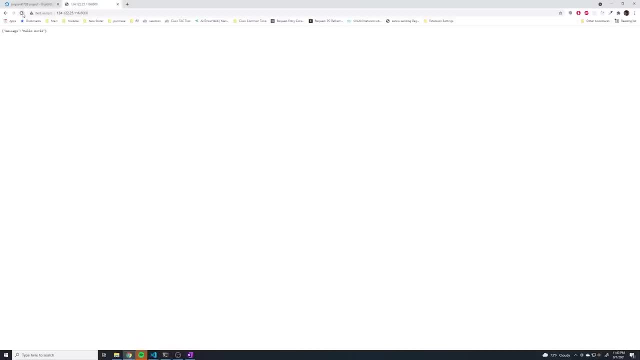 Now you can see it's listening on any IP And we're going to refresh. And if you guys can't see that, you can see that it's not listening on any IP And we're going to refresh. And if you guys can't see that because it's tiny, we can see that I got message, Hello. 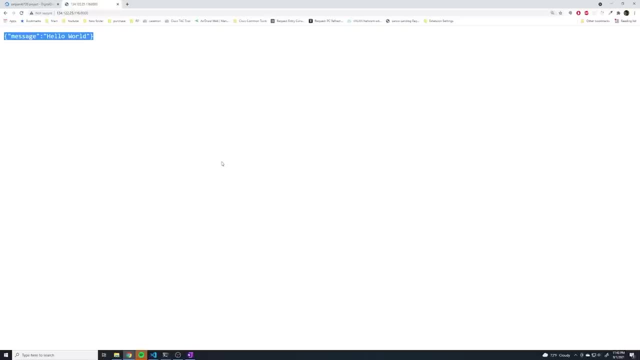 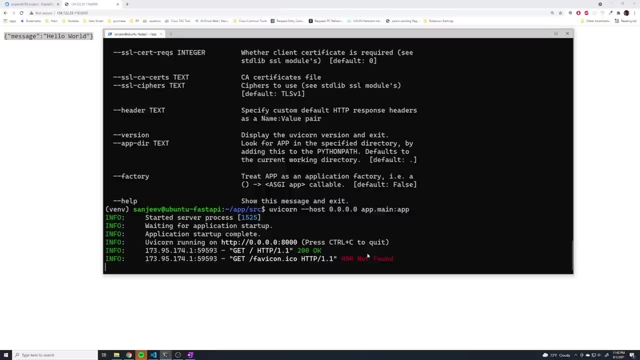 World, which is accessing that route, path that we have. So it looks like things are working at this point. However, right now you know if we, if this program crashes or if we reboot our machine, you're going to see that it doesn't actually restart automatically. 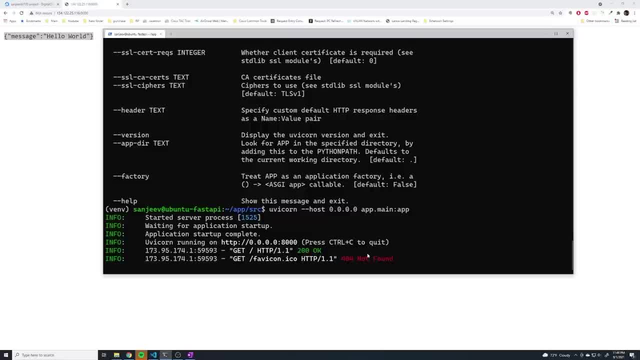 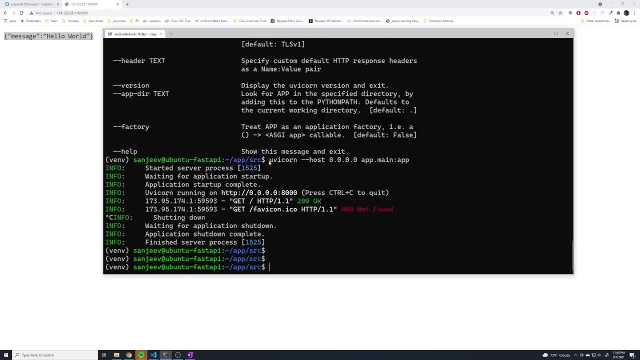 And so what we're going to do is we're actually going to use a process manager, So we're going to use something called G unicorn. So Ctrl C out of that, instead of just starting our application with UV corn, we're going to use G unicorn. 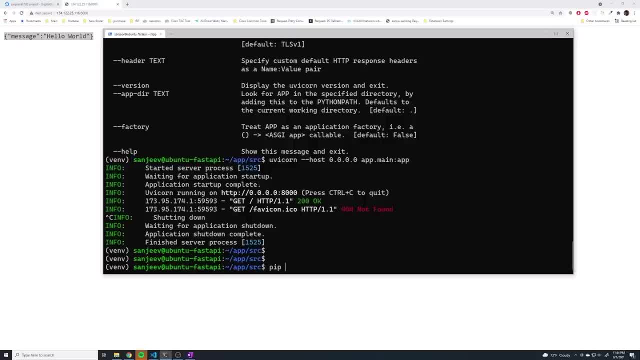 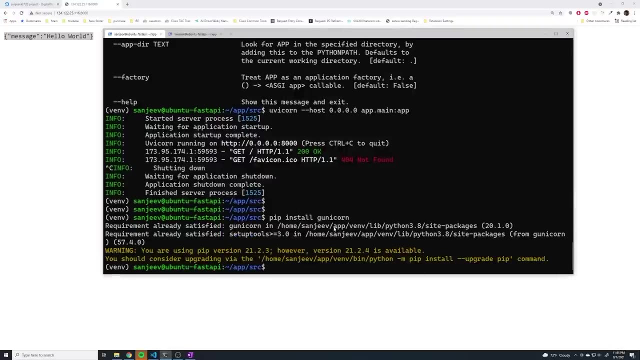 And if you don't, if you haven't already installed it, which you probably haven't do- pip, install G unicorn And make sure you're in the virtual environment, And so G unicorn is going to be responsible for starting our application. Now, I've already got this installed, because I added it to my requirementstxt file a little. 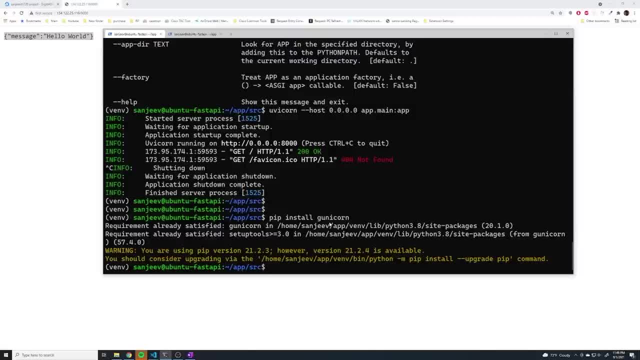 bit earlier. But if you haven't done that, that's fine, Because I haven't told you guys to do that. So just do a pip, install G unicorn And if you get any errors, most likely you'll need two other packages. you'll need pip just. 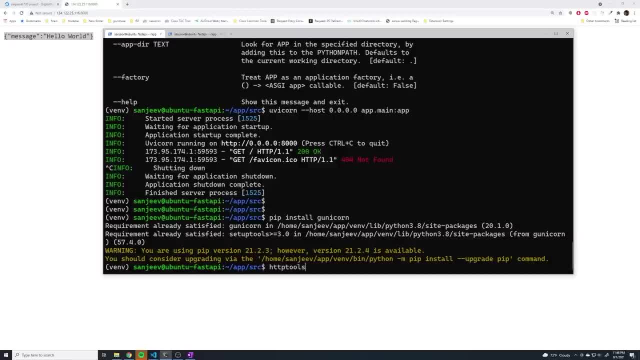 to. you'll need HTTP tools, And so you can just do a pip install of HTTP tools, And you'll also need one extra library, which is UV tools. So if you so, if you hit any other errors moving forward, I go ahead and install those two. 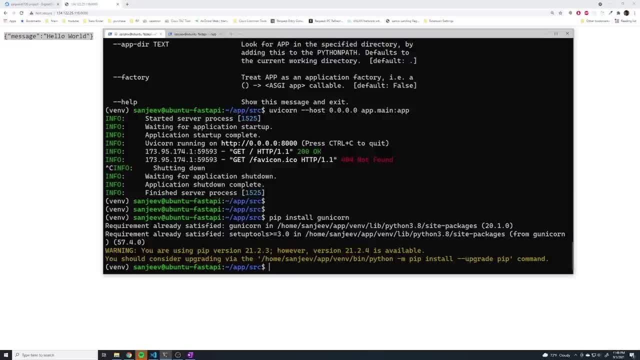 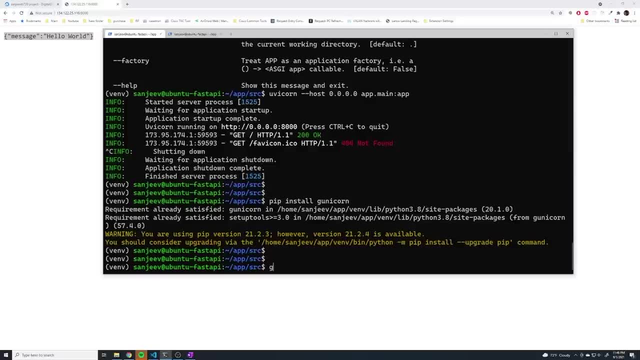 HTTP tools and UV tools, And that should fix any errors that you have. So those were some potential errors that I ran into when I was kind of doing a quick test run, But at this point we should have access to our to a G unicorn command. 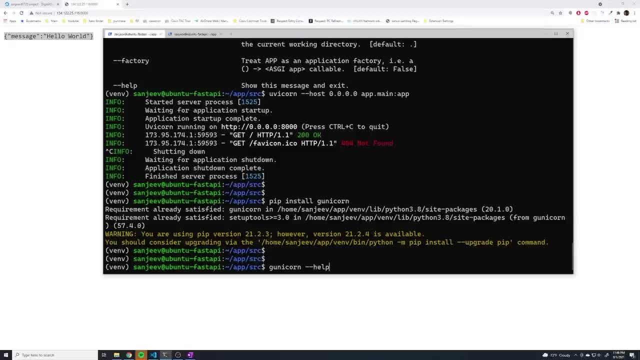 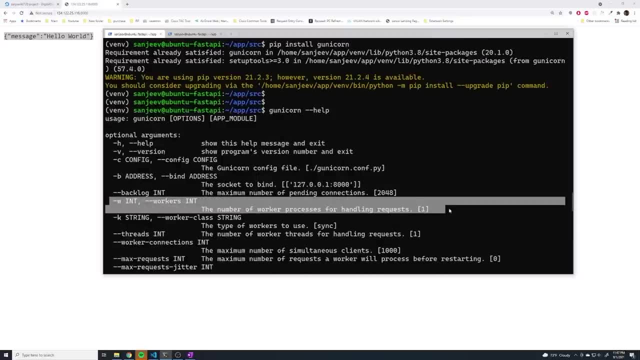 So I can say G unicorn, And let's just do a quick dash, dash, help, just to see what options we have. And here what's nice is that you can actually set the number of workers So you know if you have, if you're on a multi threaded machine or you have a virtual machine. 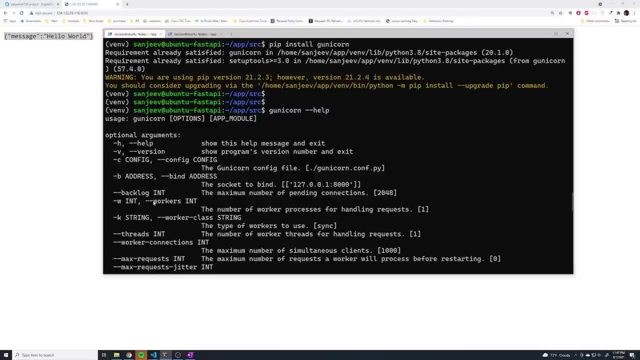 with multiple CPUs, you could set up more than one worker so that they're all listening all at once, And then it's going to get load balanced across all of them. So we're going to set up for by default, just to show you you can set up one, it doesn't. 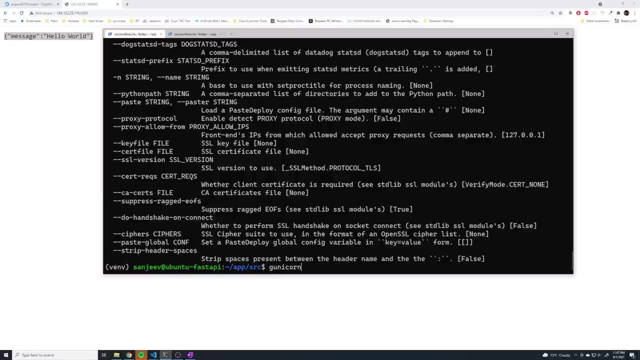 really change anything. So the command is going to be G, unicorn, dash w. So this is for the number of workers. we're gonna say I want four workers And then we're going to say dash k. we're gonna say UV, corn dot workers. 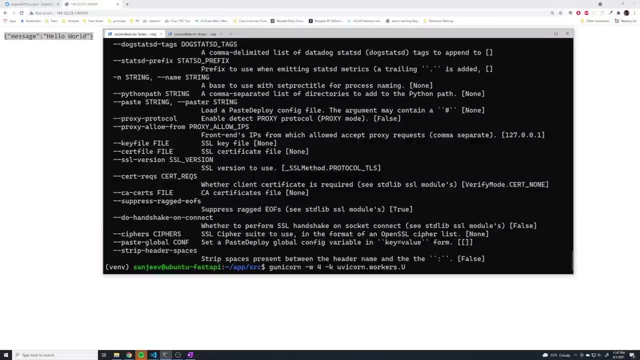 Dot capital. UV corn Capital worker. All right, and then now we just specify how to start our application, like we normally do. So we go into our app folder, we grab the main file and then we start app. And then you know, just like we did with UV corn a little bit while ago, we had to start. 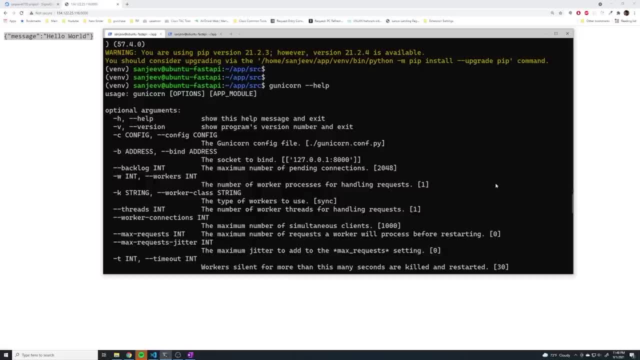 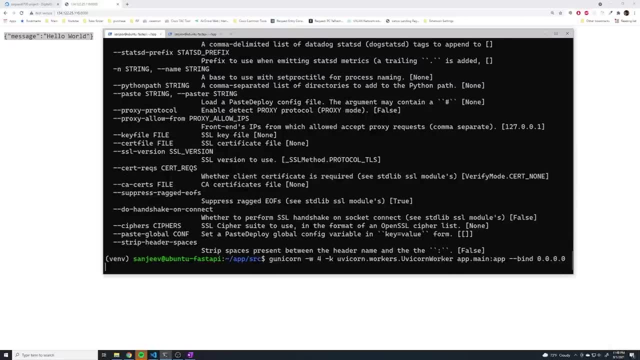 it with the dash dash host and then do all zeros Here with G UV corn- Sorry, G unicorn- we have to use a dash dash bind And then we do 0.0.0.. And then we specify the port we want to listen on. 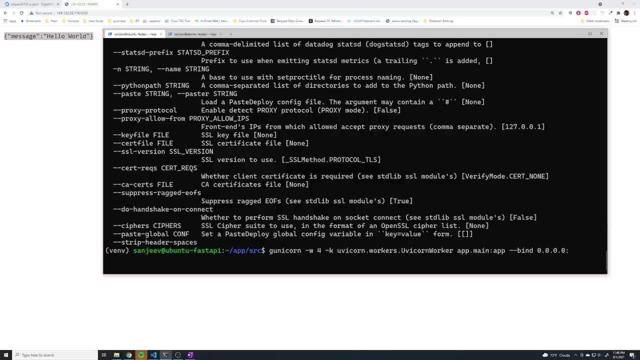 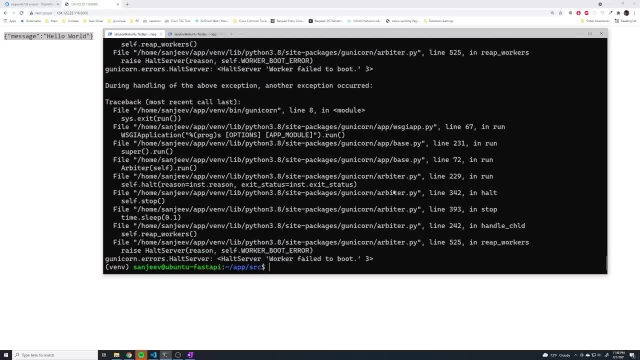 Let me drag this so it looks a little easier to read. So we do that and then the port that you want to listen on, Let's start that, And it looks like I got a couple of errors, So let's see what happened. 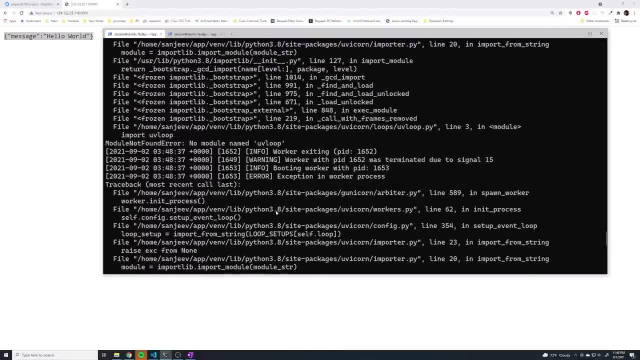 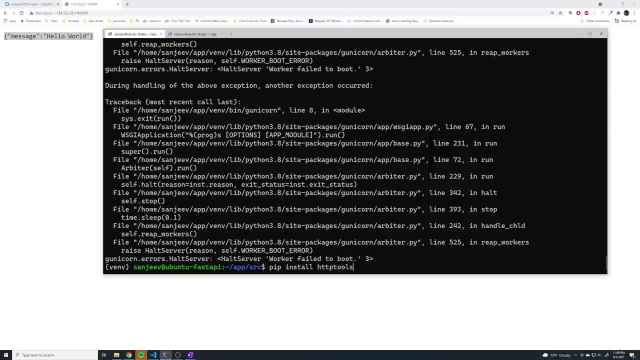 All right, And so if you get this error, UV loop, It means we're missing a library, And so, like I said, if you get any errors, make sure you do the pip. install HTTP tools. I should have this one already installed. 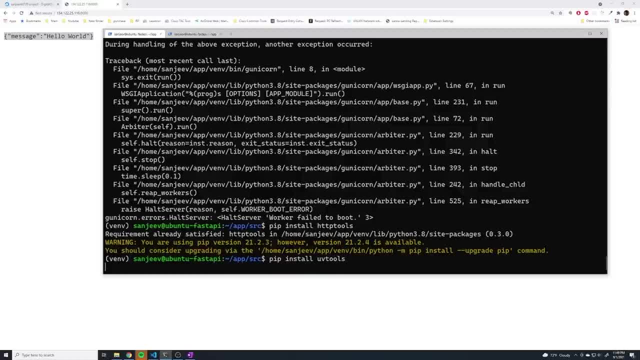 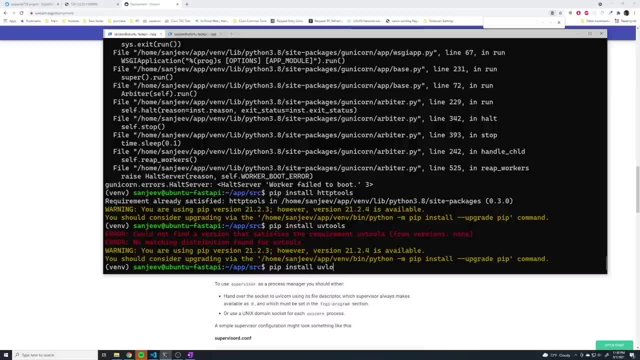 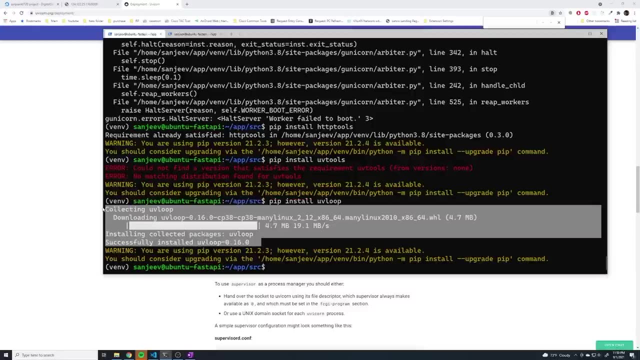 And then you want to do a pip, install UV tools, And I realized I've been making a mistake. It's not called UV tools, it's going to be UV loop, Alright, and so now it's successful. So not not UV tools, UV loop. 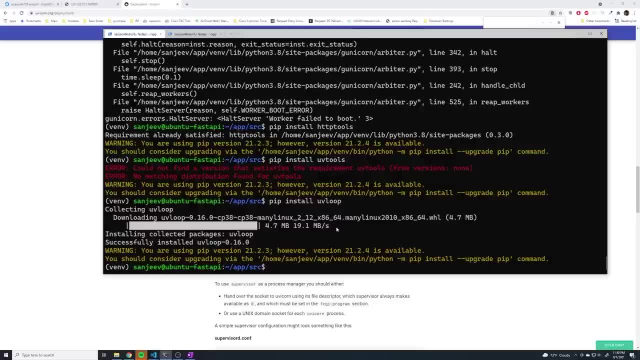 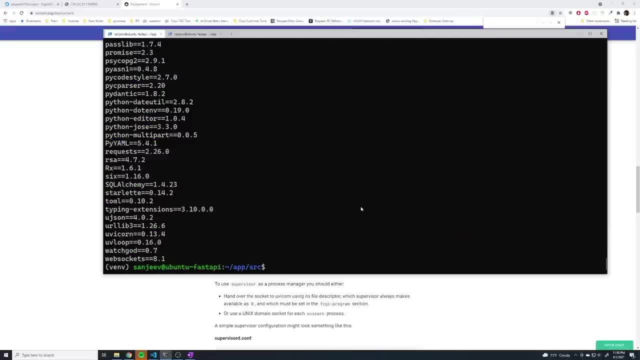 All right, I guess I got it mixed up with HTTP tools And so you can go ahead and if you actually wanted to, if you did a pip freeze, you could go ahead and copy this and make this your new requirements, that TXT file that you check. 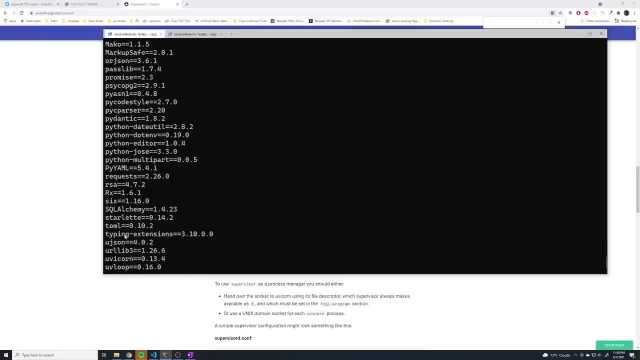 into Git. This is going to have G unicorn automatically in there, because we already installed it. It's going to have UV loop And it's going to have the what is the last one that we needed, HTTP tools, which is right here, And so you can check this version into Git. 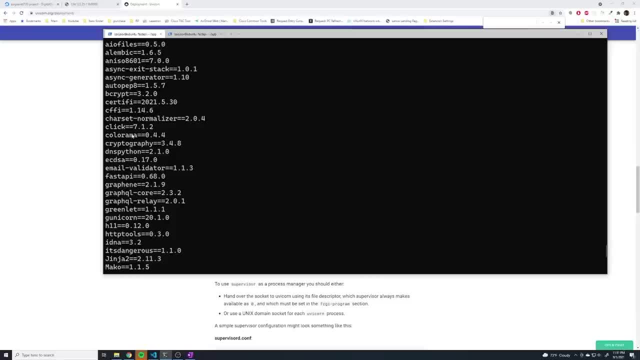 And so that way it's all up to date, And so when you deploy to other Ubuntu machines or other computers, it's going to have all of these extra packages, so you can deploy right away. Alright, and now let's run the same G unicorn command. 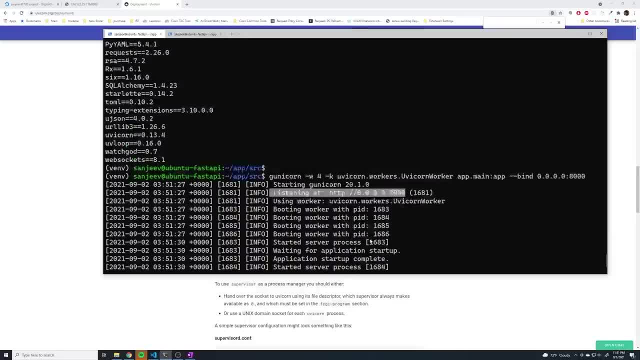 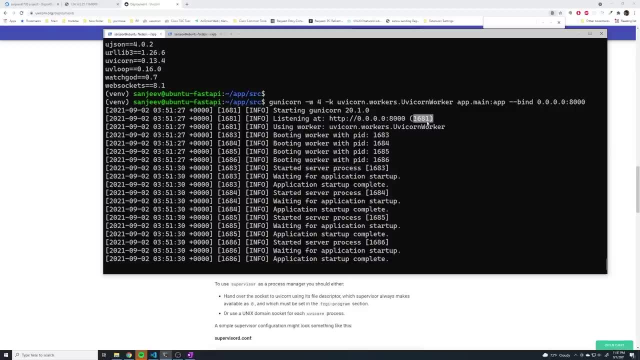 And now it looks like it started. it says it's listening on this port And notice something interesting. Look at this. it actually started up for worker nodes and you can even see the process IDs. So this is probably the parent ID And then these are the little worker IDs. 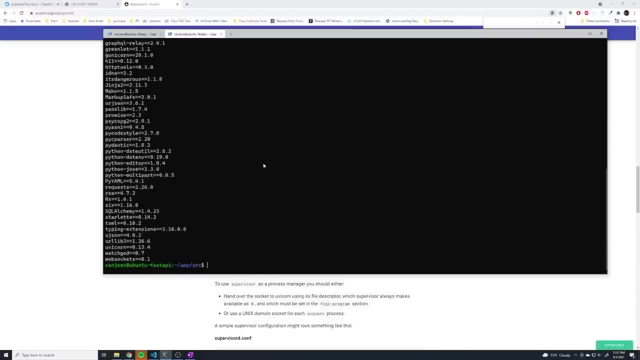 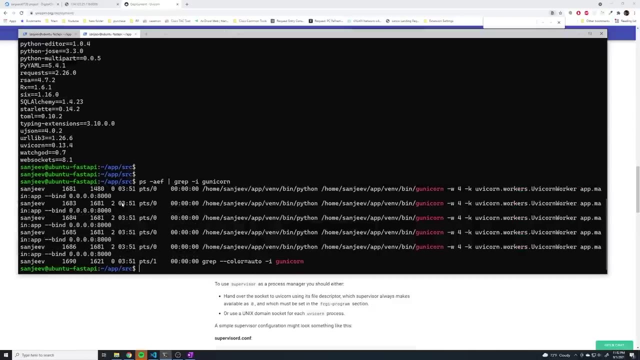 So if you wanted to, we can open up another connection And I can do a PS dash, AF pipe grep. We can probably just grab for you G, G, unicorn, Yep, And so you can see all of the different processes that were started. 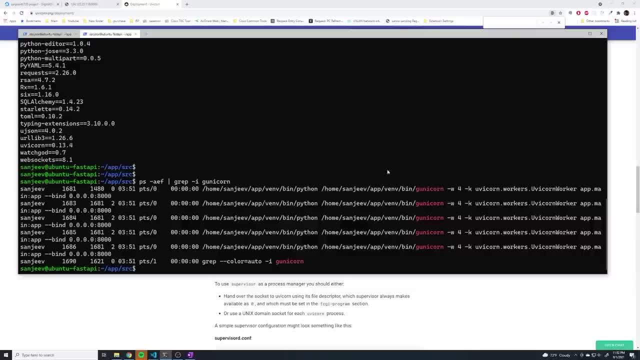 And so there should be five of them, 12345.. One of them is the parent process and then the four are the other child processes. Right now, that's working. Let's just do a refresh, just to make sure we didn't break anything. 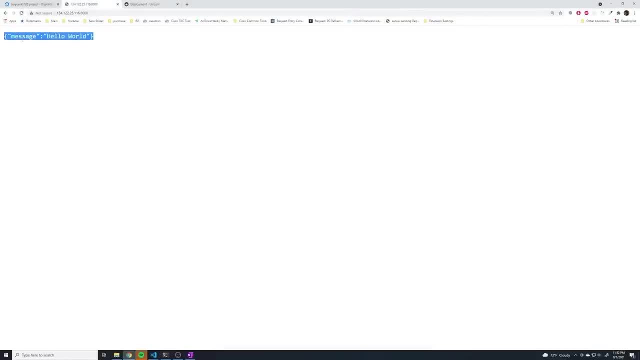 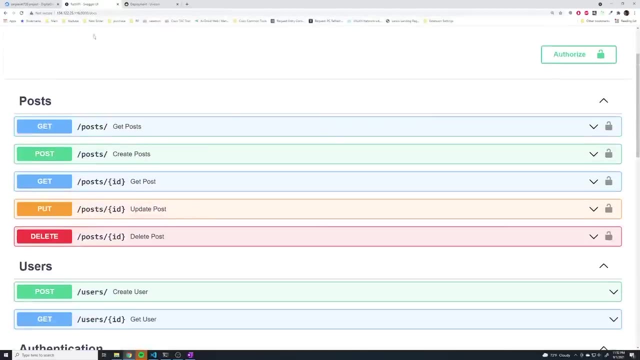 And it's still working, And so if we do a refresh, you can see that we can still access our application, And if I go to slash docs, the documentation should still be there. Perfect, So it looks like our app is working. we can test it now by testing the individual endpoints. 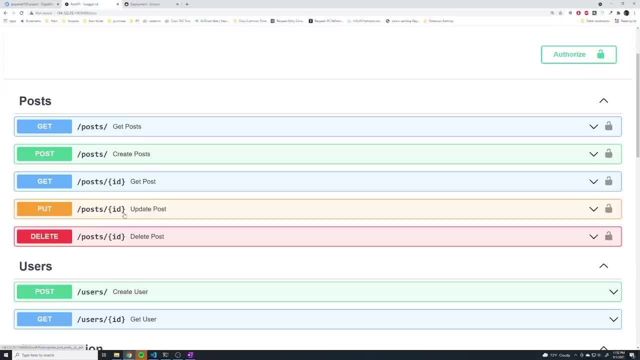 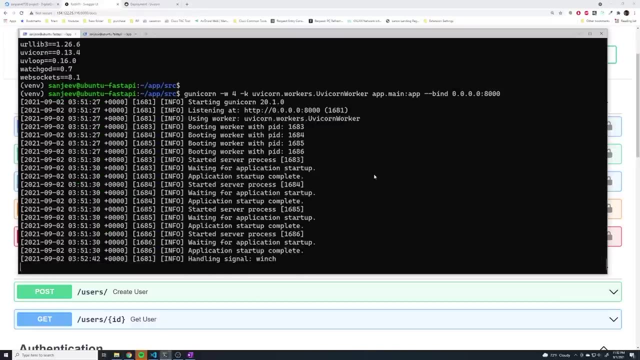 But we're going to hold off on doing that because we're going to make a few more changes. So the first thing is right now. this is: this is running on our specific terminal, And so it kind of locks up our terminal. 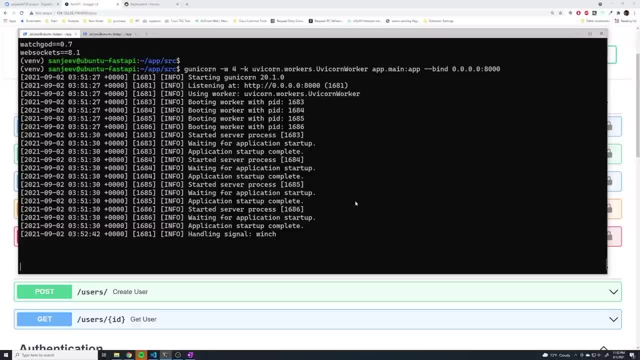 I want this to be running in the background And, more importantly, I want this to automatically start up on boot, because right now, if we reboot our box right, we'd have to manually log into this device and run the same command. So we have to find a way to kind of automate it so that upon reboot it's going to run. 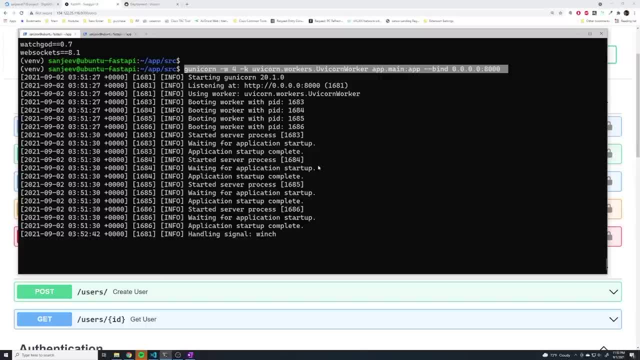 the application and we want it to run in the background so that we don't see any logs, by default, And we'll tackle that in the next video. Okay, so in this video we're going to figure out how we can have this. 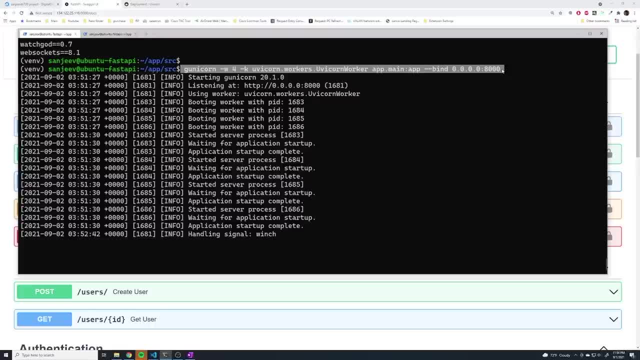 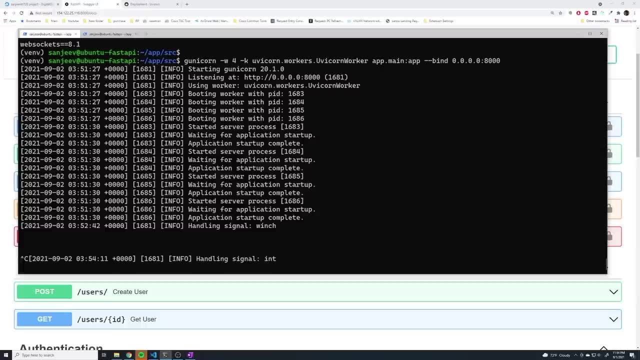 command automatically run upon reboot, as well as how can we run this as a background process so that we don't hang our terminal? So what we're going to do is just do a Ctrl C to stop it for now, And we're going to. what we're going to do is we're going to create our own service. 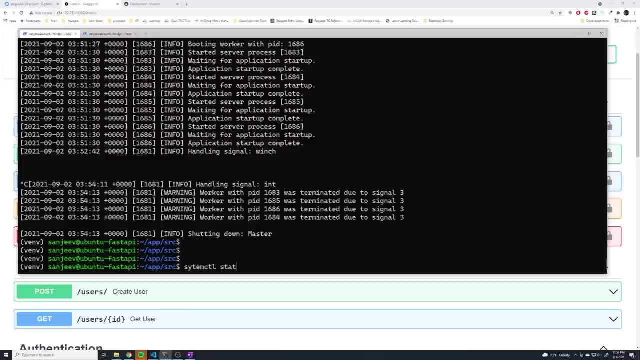 And if you ever run system CTL and then you know either status or start or or restart and then the name of some of some application that you wanted to run, You know that is going to run. That is an example of making use of a service. 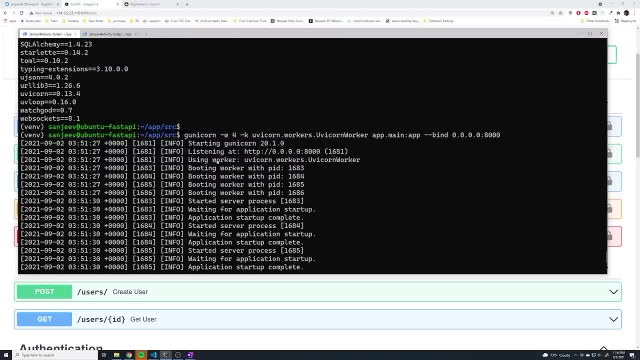 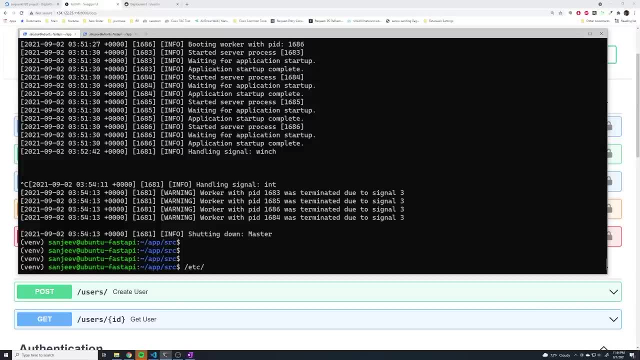 And so what we're going to do is we're going to create, we're going to make our own service which starts this application here for us, And you'll see that it's actually pretty simple If we go to slash Etsy, slash system D and then system, and I forgot to do a CD to move. 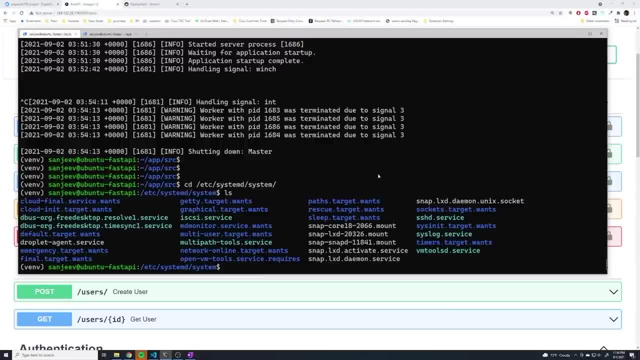 into that directory If you do an LS. these are all of the services that have been installed on our machine And we're just going to create a brand new one. So how do we create that? We have to create a couple of files. 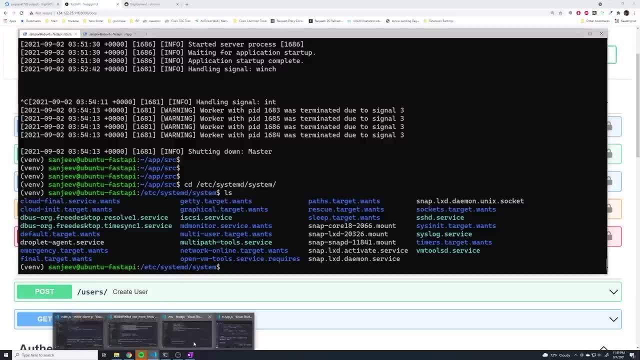 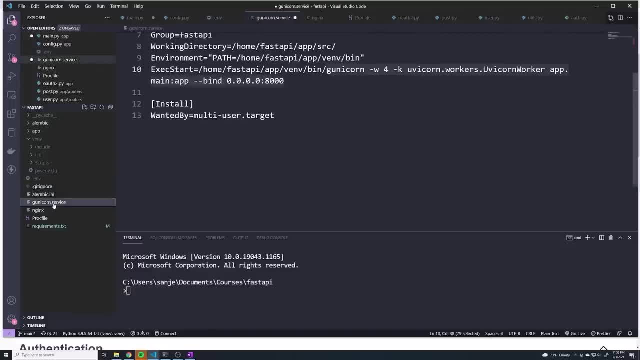 And I have actually created them for you guys ahead of time. So if you check my GitHub repo, you will see a file called G unicorn dot service And there's going to be a couple things that we have to change. So let me just walk you through what each one of these lines mean. 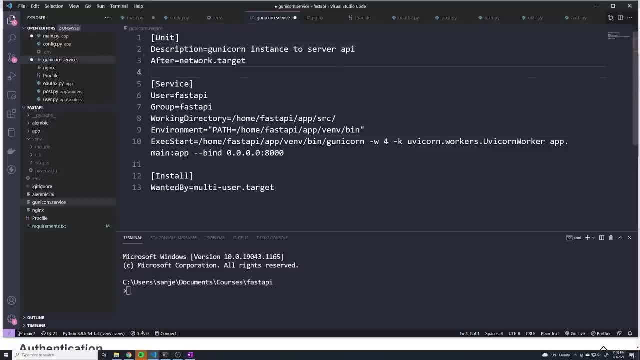 So under unit here we're just going to give you a description of what this is going to do. So this is going to be a G unicorn instance for to server API. you can put whatever description you want. You can say: they demo fast API. 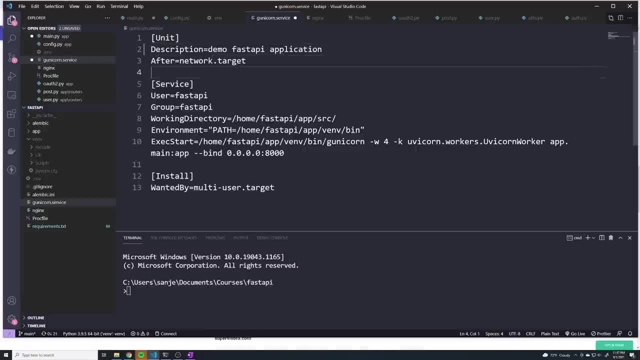 Application doesn't really matter. After now the next line right here where it says: after network: dark target. what this is going to do is this is going to tell system D or Ubuntu machine when to actually start this service. And so it's saying that, hey, we need our network service running before we can start. 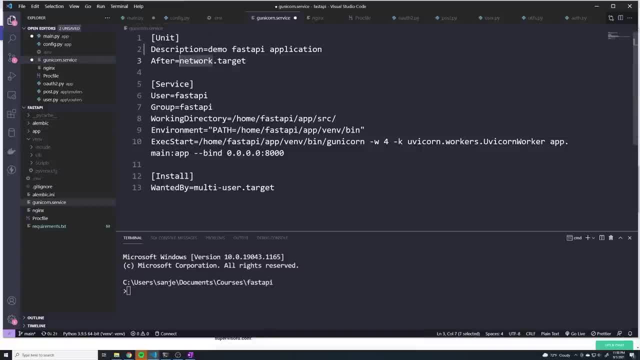 our API, because if the network's not up, then nothing else really matters. So we're going to wait for network to come up before we start the service. Then, on the service, we're going to figure out. we have to specify what user is going. 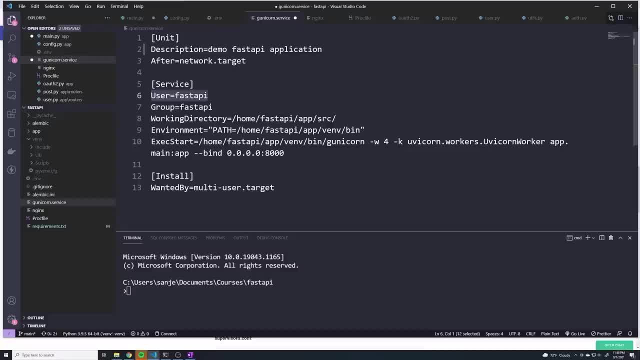 to. you know run This service, So we need this to be associated with the user. I created a user called Sanjeev, So I'm going to update this And then for group you want to just put the same exact name as the user. then we have. 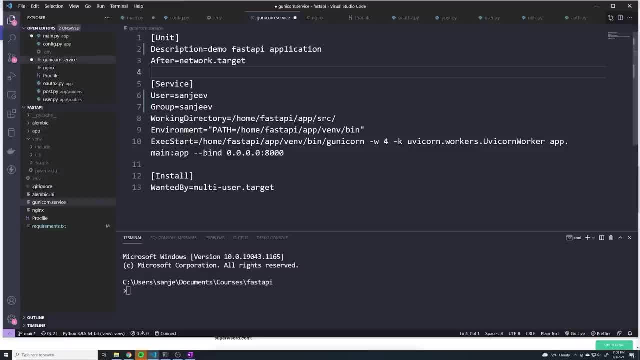 to specify the working directory, And so this is going to be the directory our service is going to be launched in. So go ahead and update this to point to the directory your app is running in, And if you don't know what that is, remember just go home. then move into apps. 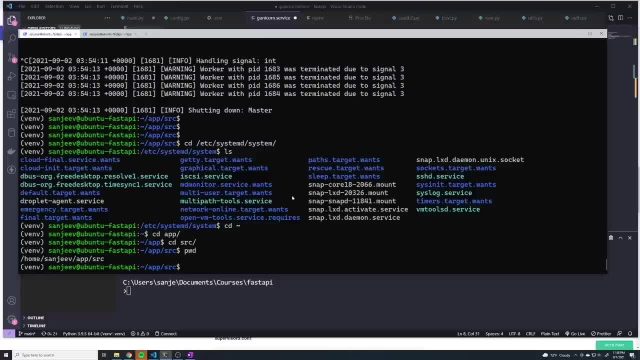 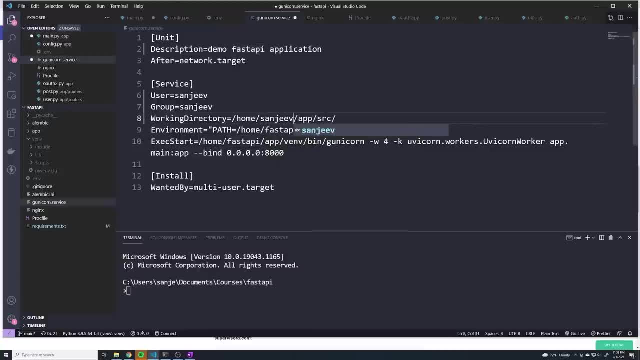 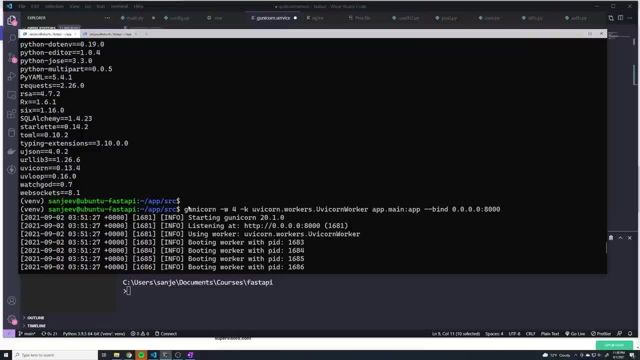 And then you can go into the source folder if you want And just type in pwd. So that's going to get you the exact path that you want, And so I have to update this with my username And then the environment. So because we want this service to run the G unicorn command, which is right, here we 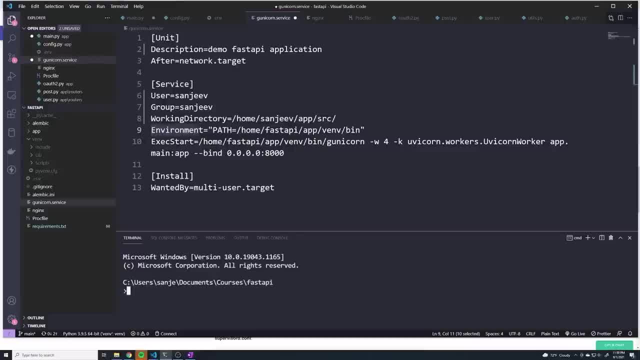 needed to run in a virtual environment. So to actually set the virtual environment through this script, we have to say environment equals and then we set this path variable And we just point it to the exact path to our bin folder. So once again, you don't know how to get there. 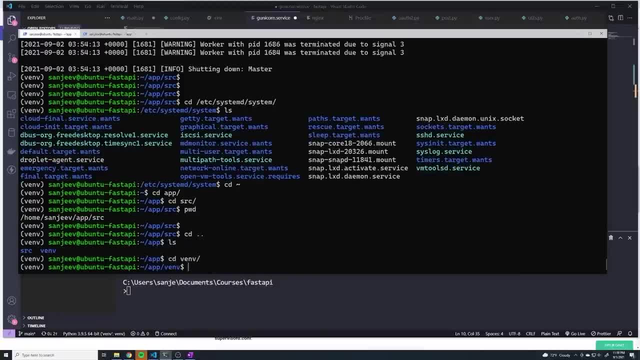 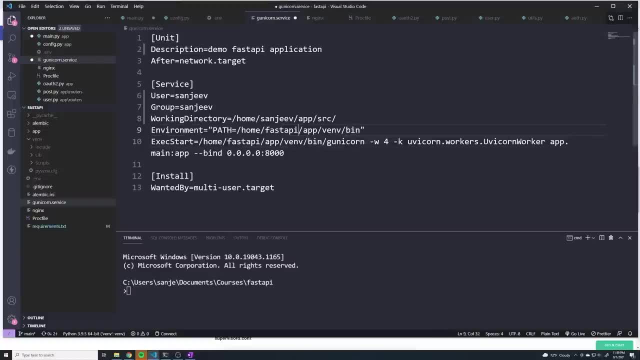 Just go to your app folder, go into your virtual environment, go into your bin folder and then just type in pwd And that's going to get you the path. And so I just have to update this with my username And you'll just do the same thing. you just have to update the username, then we have. 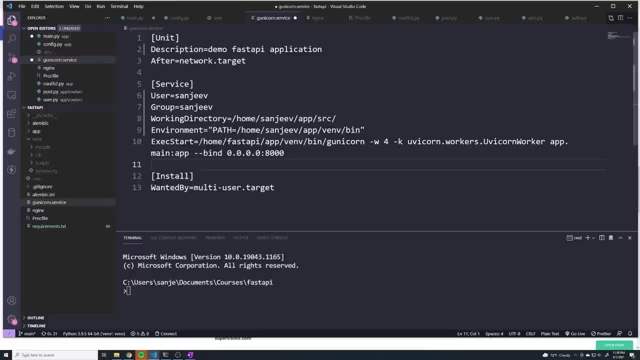 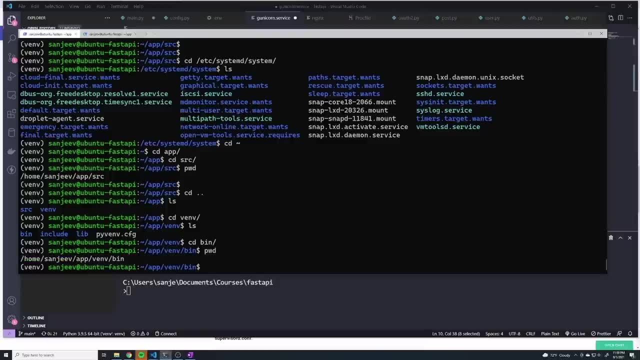 to specify the exact command to run. So we have to provide the path to where the G unicorn command resides on, So it actually sits in the bin folder. So if you actually do an LS here, Right, you can see the G unicorn command. 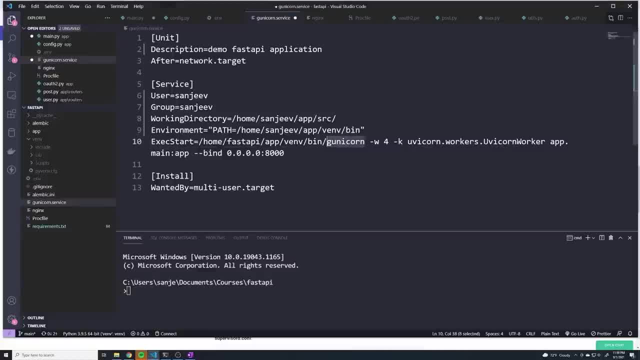 And so that's going to give it the path to the command. And then after that- well, actually I have to update my username once again, And after that it's the same exact command that we ran for. So for workers, dash k, then we have this long command right here. 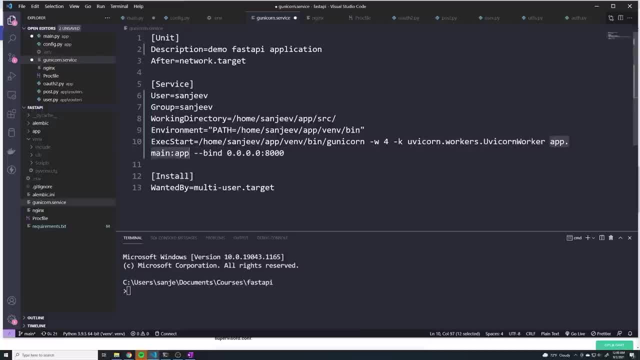 And then we specify how to start our application, which is this command, and then we're going to bind it to 0.0.0.. And then you can pick whatever port that you want, And this is just a default config. You don't have to worry about it, you need it. 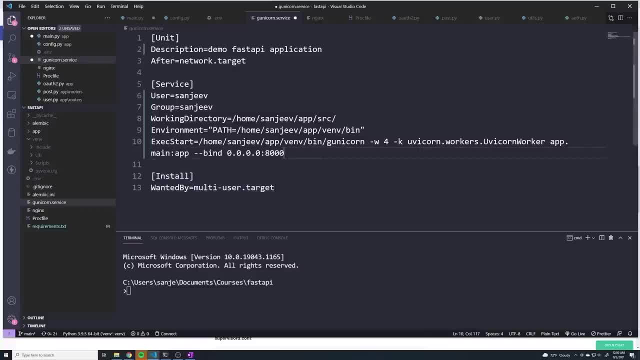 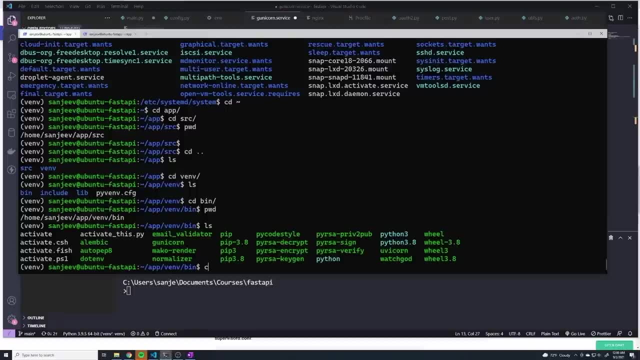 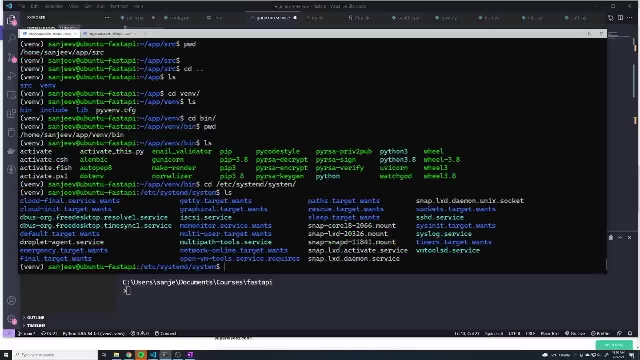 But I don't want to go too far into how Linux works to actually explain this. Just know that this is just a standard procedure for creating a service. So to actually create the service Now, what we do is let's go to slash Etsy, system D, then system. 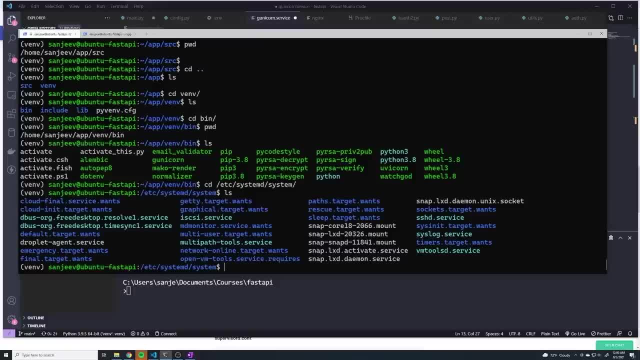 And let me deactivate my. we don't need to deactivate, it's fine. We're going to create our service file here, And so I'm going to do a pseudo VI, And then this is going to be a service file, And then this is going to be a service file. 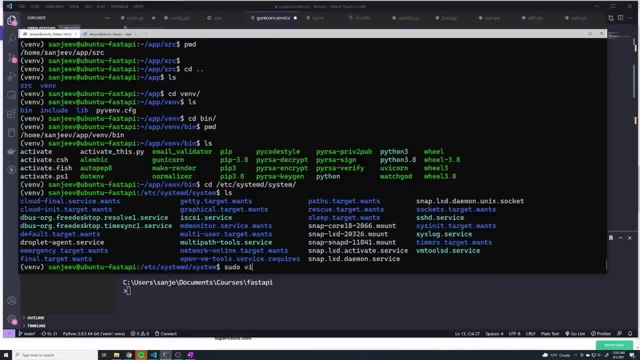 And then the name of the service. So what do you want to call your service? So when you type in system CTL and then start what's the name of the service you want to type in, you get to specify. I'm going to make it so that it's just called API. 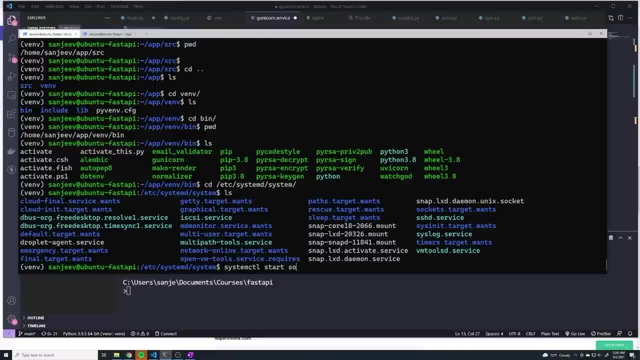 Very simple. You can call it fast API, you can call it social media app, it doesn't really matter, it's up to you, But I'm going to call it API. And since I want to call it API, I'm going to create a file called API dot service. 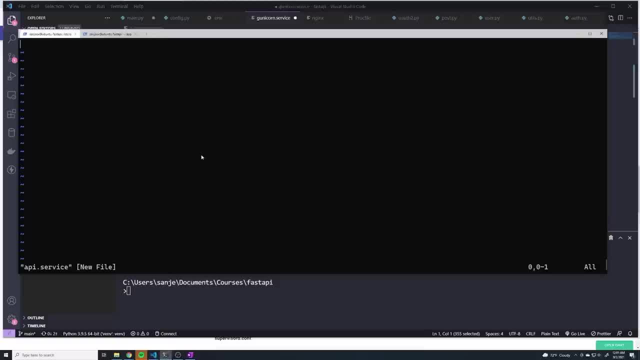 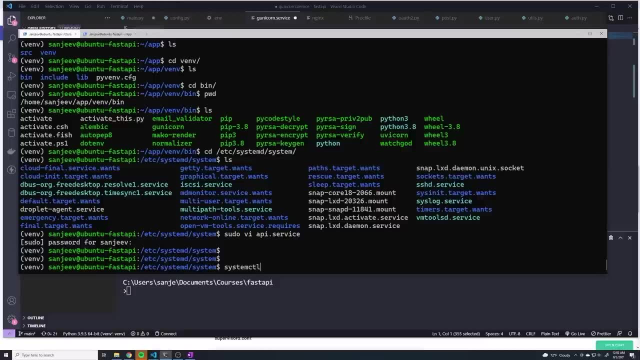 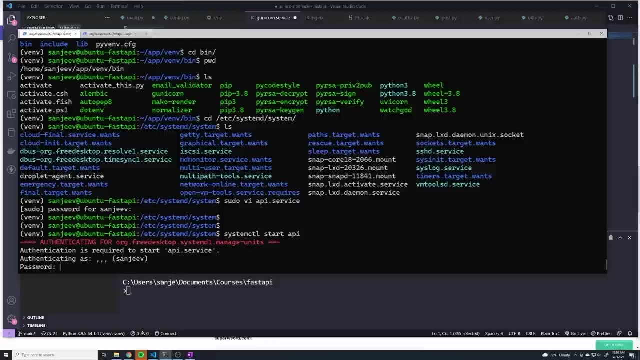 And then what we can do is just take this, copy it And we will paste it in here. Alright, and to test out our service, let's do a system- CTL Start API- And we're gonna have to put in our password. 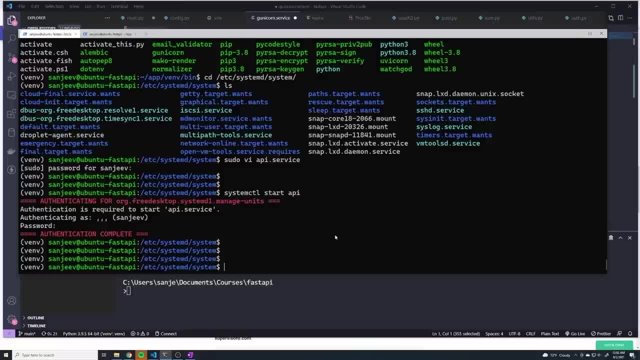 And so this started our API. And if we do a system CTL status API, whoops, there shouldn't be a space CTL status API. this should just give us the status of our service. we can see that looks like it failed. that's not good. 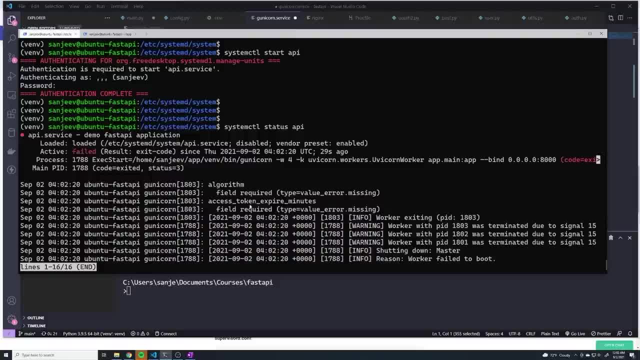 And it's going to provide us some logs And if we take a look at the logs you can see algorithm: field required. access token expires. field required. So it looks like something is wrong with our environment variables, because we saw the same exact error when we were originally setting this up, before we got the environment variable. 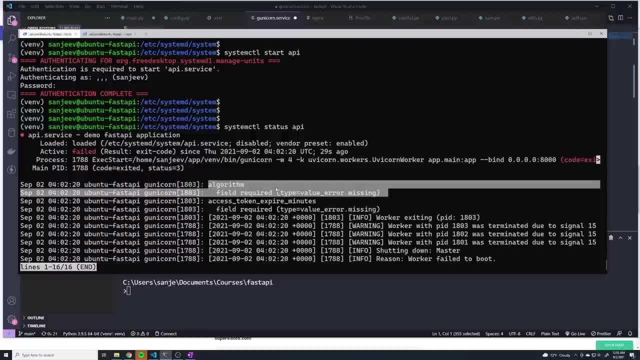 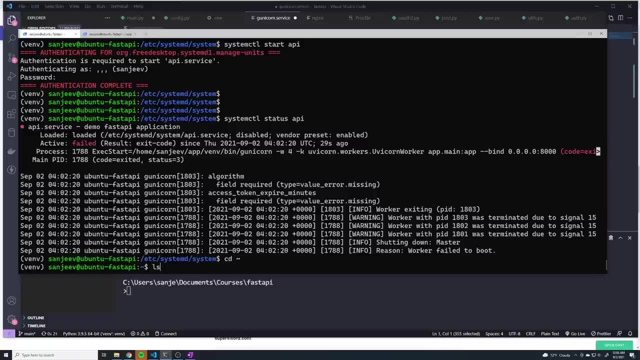 So for some reason it's not actually accepting these environment variables, And the reason for this is that the service file, the service that you create, doesn't have access to users environment variables. And if you actually go back to our home directory and then we go to ls, ls minus la remember. 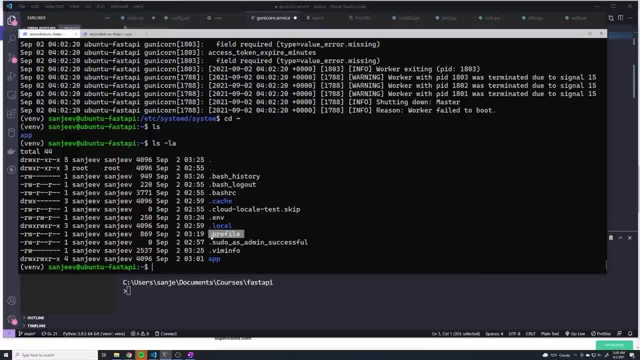 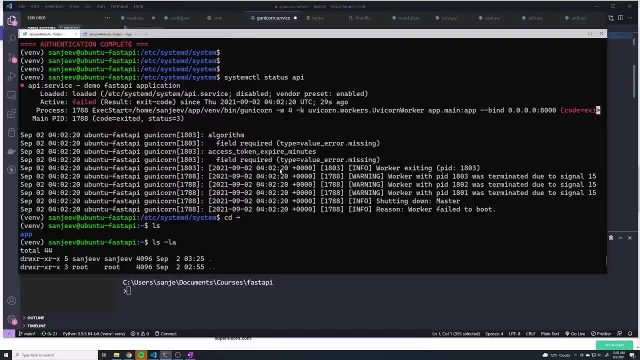 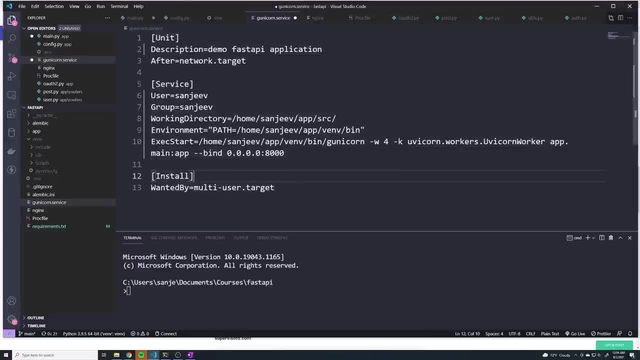 we created this ENV file and then we loaded it in the dot profile. So the environment variables that get loaded from dot profile aren't accessible within a service, And that's just the way services work. So what we have to do? What we have to do is we have to pass in another field in our service config so that it knows. 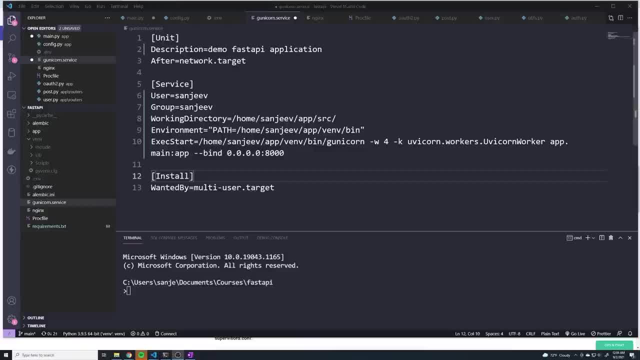 to pull the environment variables from that specific file. So what we can do here is in this file we're going to go and just add another line. it doesn't matter where you add the line, But we want to say environment file. make sure to capitalize the E and the F equals. 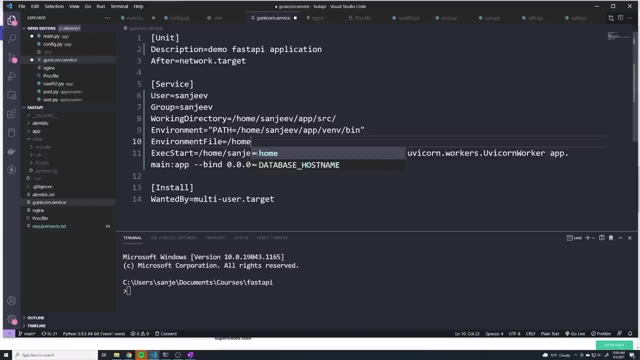 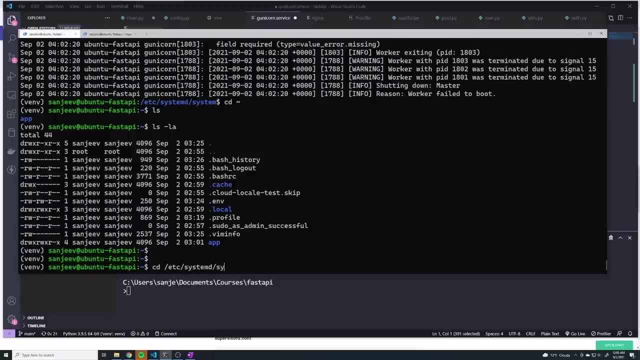 and then you provide the path to your specific E Ah Env file. so mine's gonna be home slash Sanjeev dot Env And I'll just copy all of this again And we'll go back into Etsy system, the system. 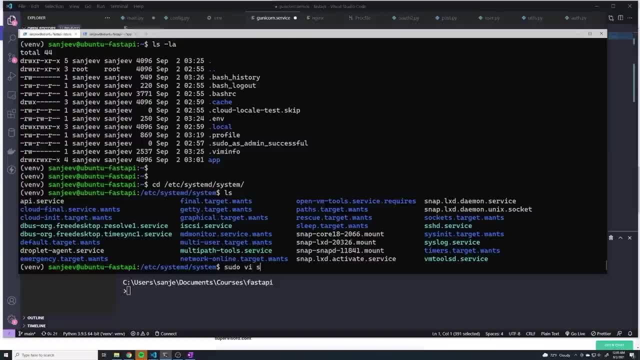 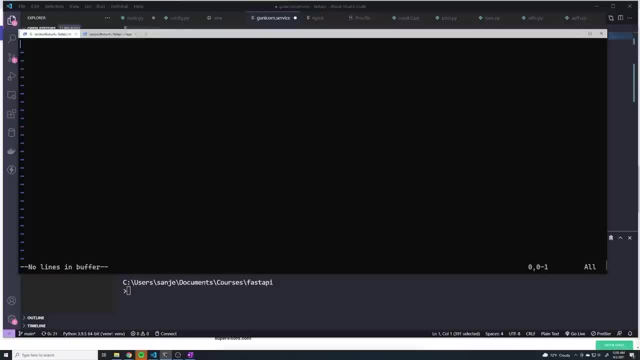 And then I'll just do a sudo vi API dot service And we're gonna replace this file now. Alright, so now we should be able to import all of those environment variables. And you, there's other ways to do this. you can also set up a config file for your, your new service. 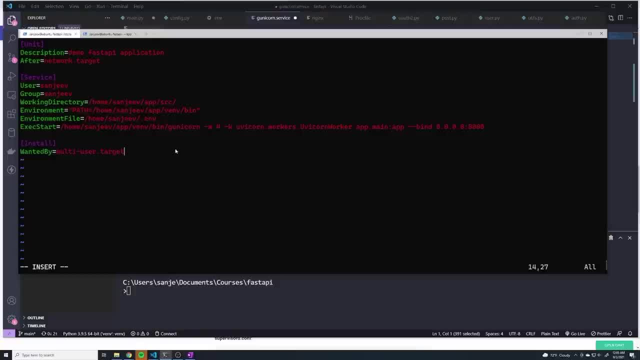 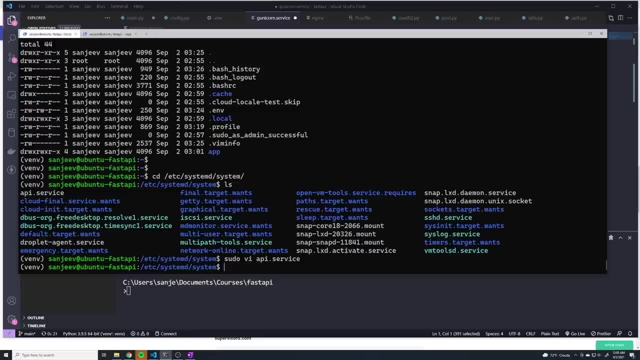 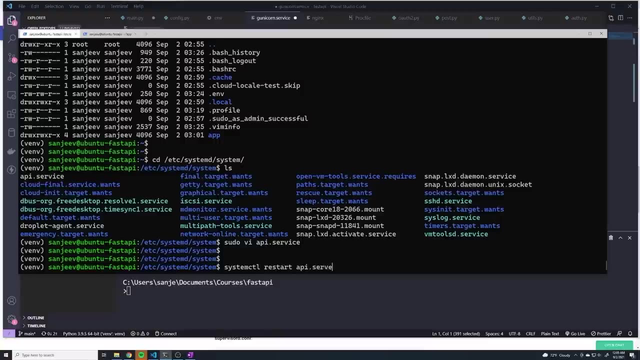 However, I figured it's just easier because we already have our environment for our, our dot ENV file, So we can just continue to use that. And now if I do a system CTL, restart API And notice you don't have that type in API dot service. It's optional. you can you. 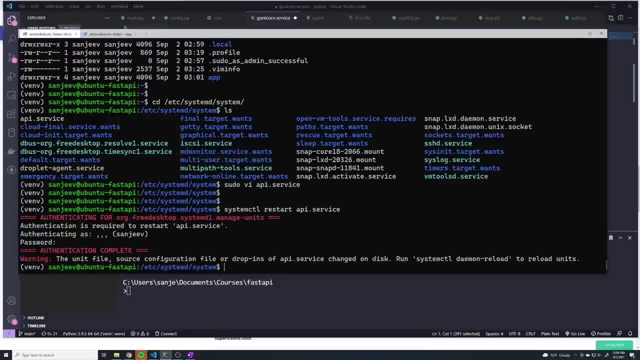 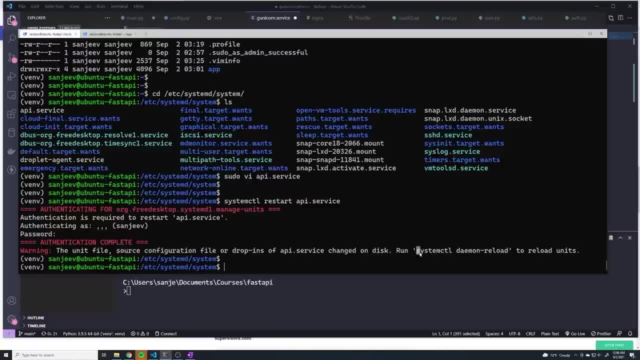 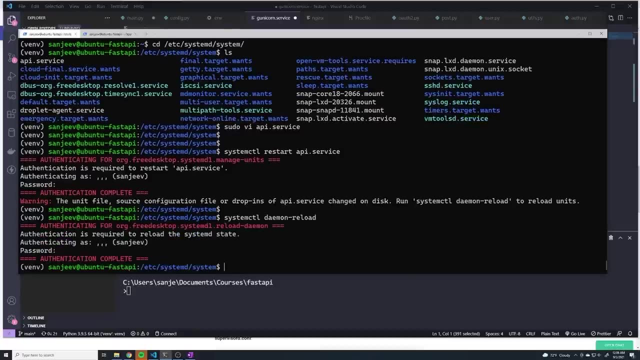 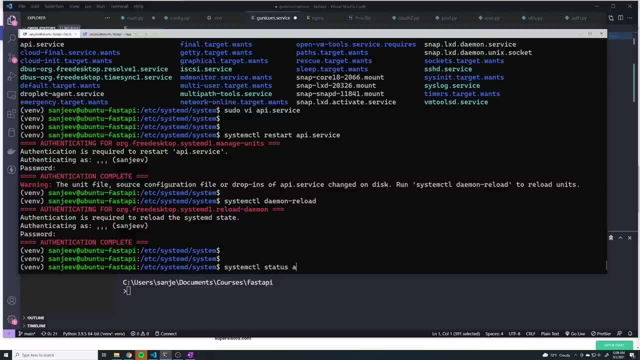 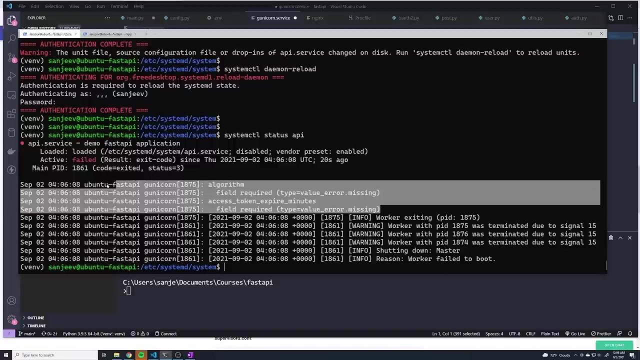 can technically do it like this, And it looks like, since we actually changed the file, we have to run this command now. drugs, All right, and so now let's do a system: CTL restart Start now ऊ restart status API. And uh, looks like we got the same exact error. Let's just do a. 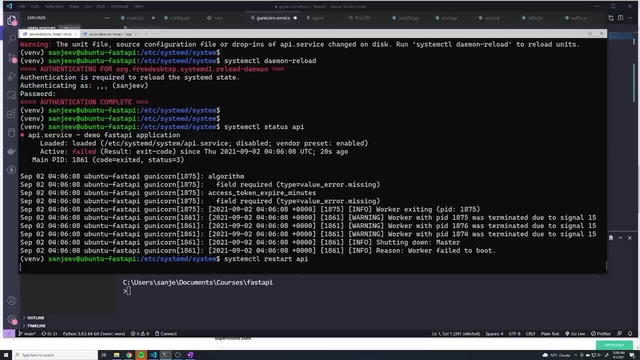 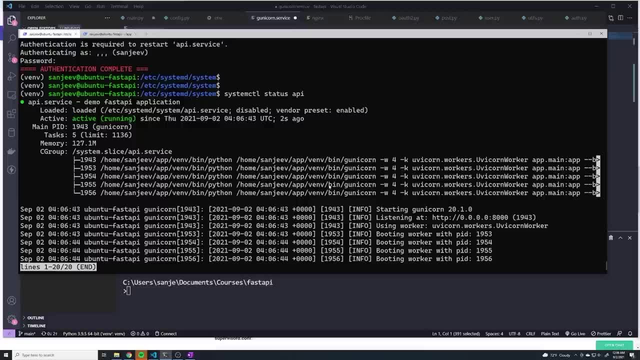 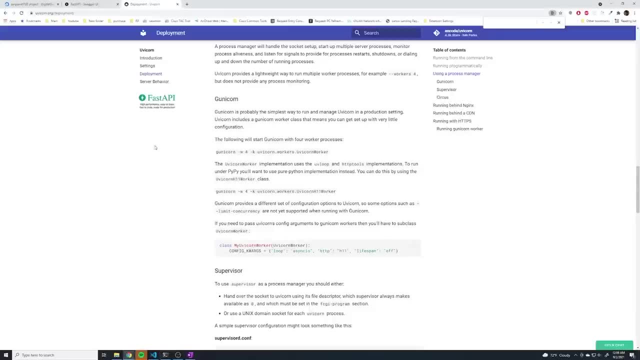 restart one more time And we'll do a status. And now it's up and running. Perfect. Look at that. So we've got our four workers. These are the process IDs And let's just double check and make sure that we can access our specific website. So I'm going to just refresh. 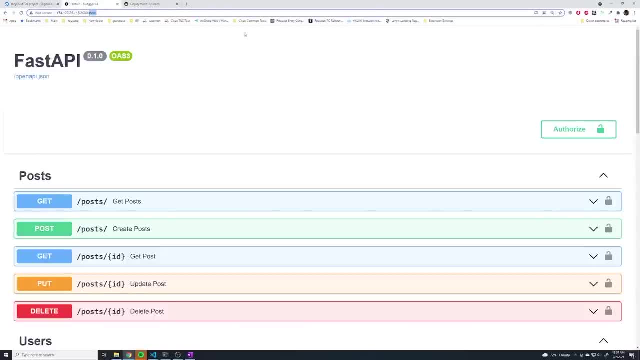 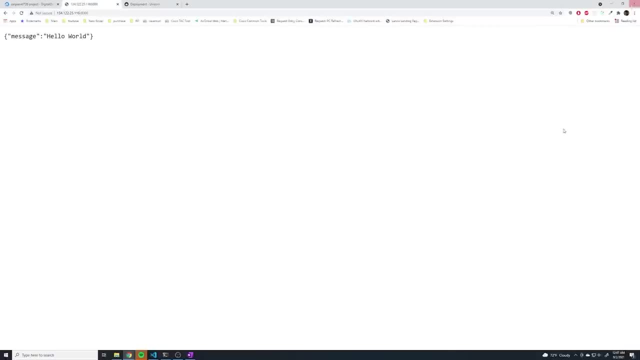 on the slash docs And it looks like it works. Let's go to the root And let's go to the root URL. I'll just change this to the root URL and see if we get the API response. Perfect, So it looks like we've got our application up and running. There's just one last thing. 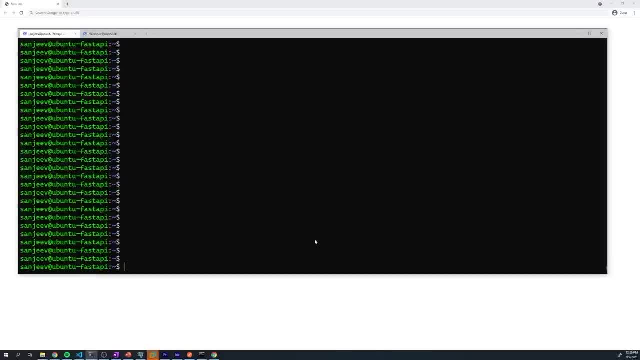 we need to do, And I wasn't sure if I had already covered this. But there's one last thing I want to do, And that is I want to make sure that our service automatically starts upon a reboot, So that way you know, in case our machine goes down, whether it's because of a power failure or 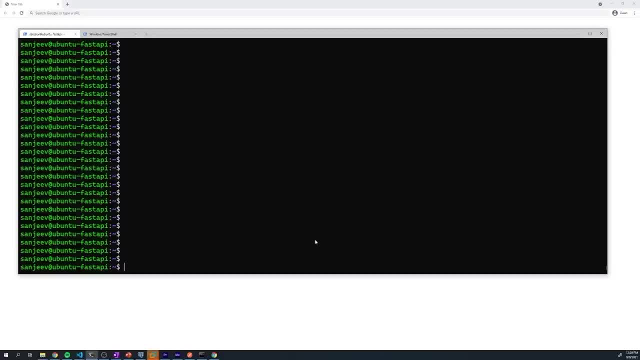 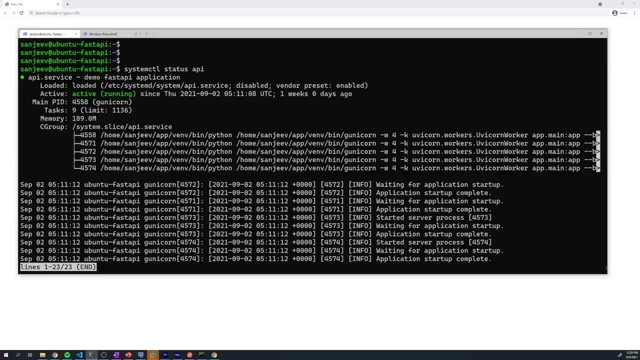 something like that, or maybe we perform some sort of upgrade. I wanted to automatically start this service so that our application is always up and running. If you do a system CTL status API, you can find out pretty easily whether this service is going to get started. 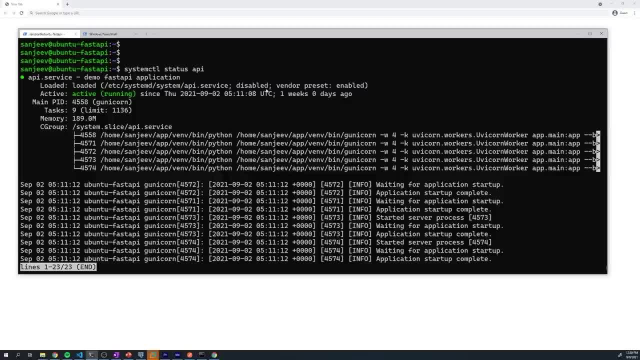 upon a reboot. So if you take a look right here under loaded, and then right here is the keyword that you're looking for, And then if you see disabled right here, that means that it's not going to automatically get started upon a reboot. if you see it's enabled, that means it will automatically. 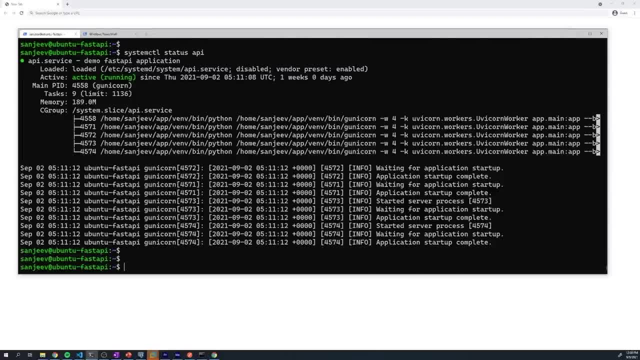 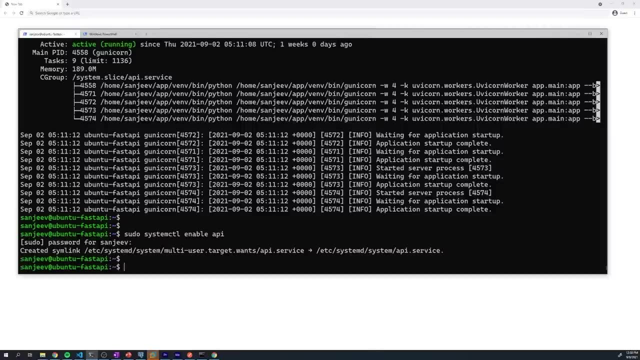 get started upon a reboot. So to actually make sure that it actually does get started upon a reboot, just do a pseudo system, CTL enable, and enable, then the name of the service, which is API, And after that, if we do a status again, we should see that it moved to enabled. 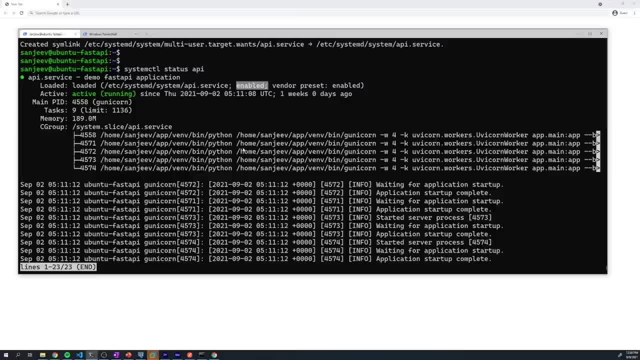 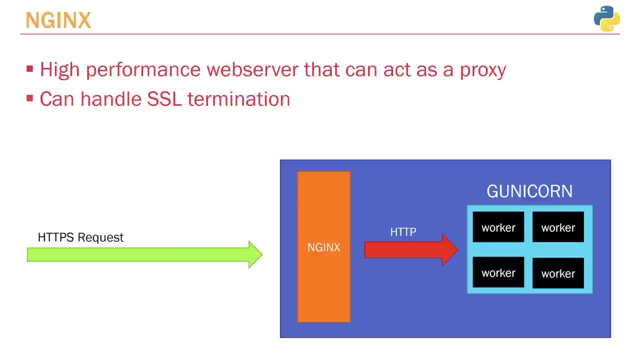 And so now, if we reboot our machine and you guys can go ahead and test this, you'll see that it automatically starts up the service. Right now, the way that we have our deployment setup is that when we send a request to our server, you know, to the specific IP address of our server and whatever port we decided- 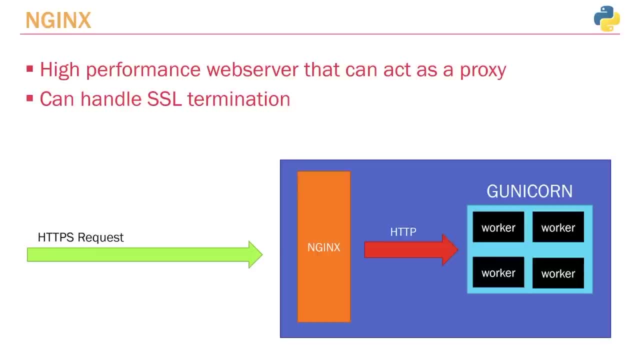 to configure our app to listen on. we send that request directly to the app or G unicorn in general, And this is technically perfectly fine. However, you'll see that in more professional type deployments, what we'll have is a intermediary web server, So we'll have a web server running on. 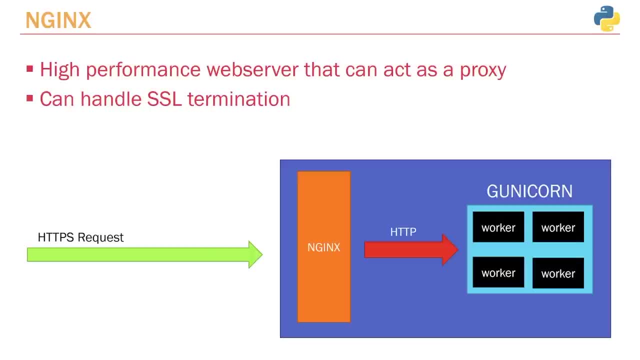 our Ubuntu machine, And that web server will receive the original request and then act as a proxy and proxy that request to our specific application, or G unicorn in this case, And so one of the common web servers that can be used for that is NGINX. There's a couple others like. 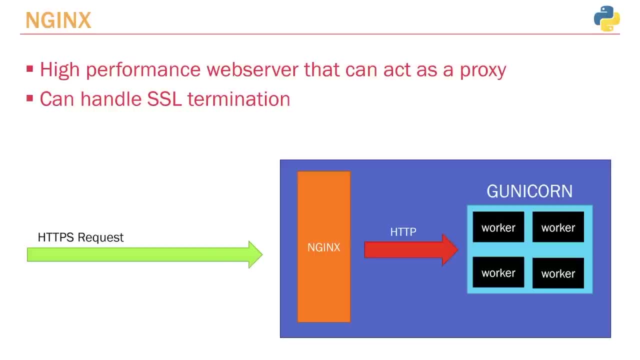 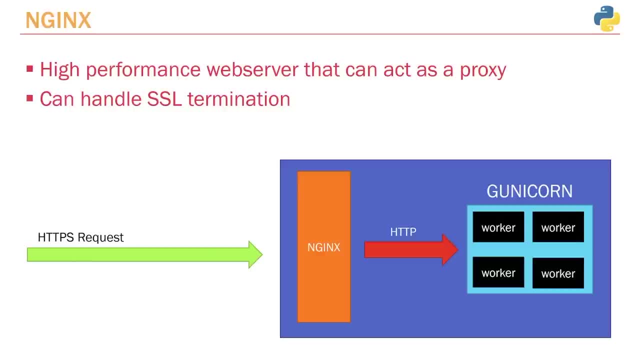 a web server that can be used for that. So you can have a web server that can be used for that. So this, or configuring our application ultimately to be deployed like this, is that NGINX is optimized for SSL termination. So NGINX is a high performance server and it can perform all of the SSL. 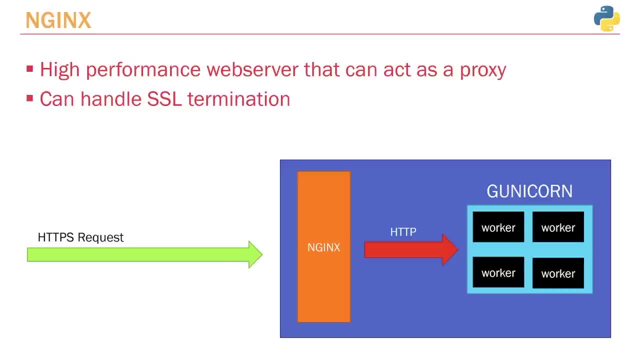 termination. So when we when we send an HTTP s request, we can send it to our NGINX server. the NGINX server can process it and then forward it as a plain HTTP packet to our application, Because technically we could configure our application to handle HTTP s. it's not optimized for that. 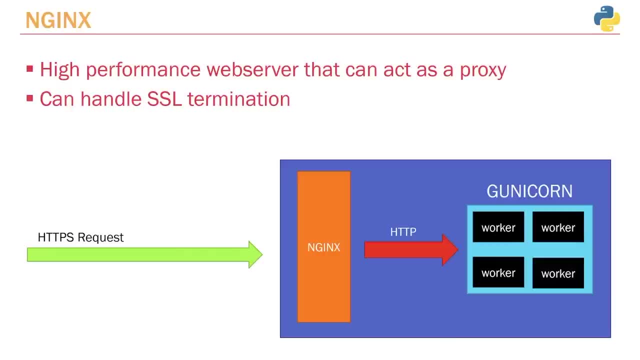 for that Right. our, our app is designed to just act as a plain API. when we start adding responsibilities like performing SSL offload, well, then you'll see that we start to see a degradation in performance. And NGINX, like I said, is a high performance web server. it's. 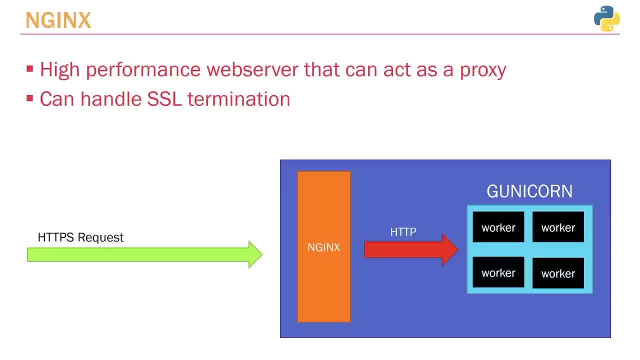 optimized for this. So it makes sense to kind of handle that responsibility on NGINX instead of our application. So that's what we're going to do: we're going to configure NGINX And this is going to act as the gateway into our system. So any request we send to our application, we're going. 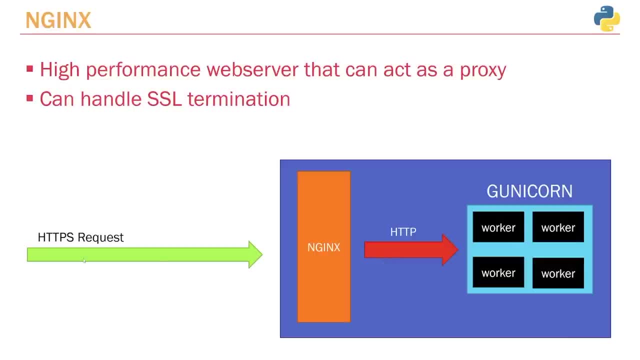 to send to our system. whether it's HTTPS or HTTP doesn't really matter. we're going to send it to NGINX, And if we send it as HTTPS, what NGINX will do is it'll then take it and send it and forward. 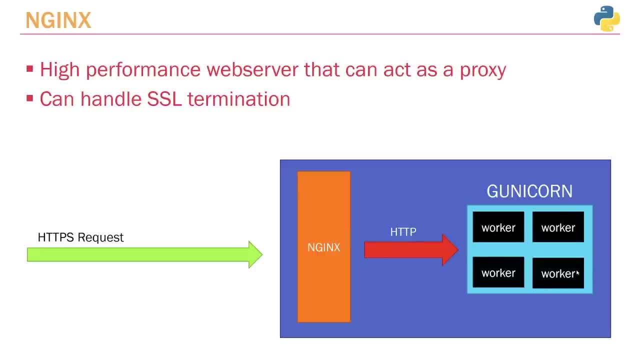 it as an HTTP packet to our application, And so I'm going to walk you through how to set up NGINX. It's not difficult. we do have one config file that we have to add, But outside of that, it's fairly easy to get this up and running. Let's install NGINX Now, to install a package we can. 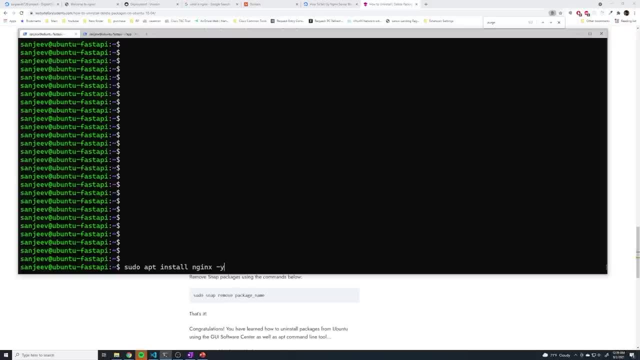 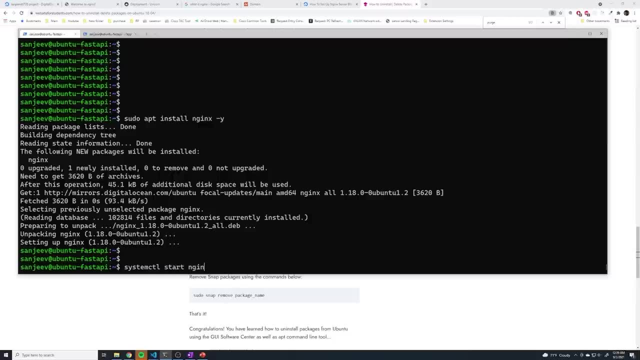 do sudo, apt, install, and then NGINX And then dash y, That installed NGINX. if we do a system CTL, start NGINX, that's going to start up the NGINX service. And so now, if you go to your server IP address, you're going to see that you. 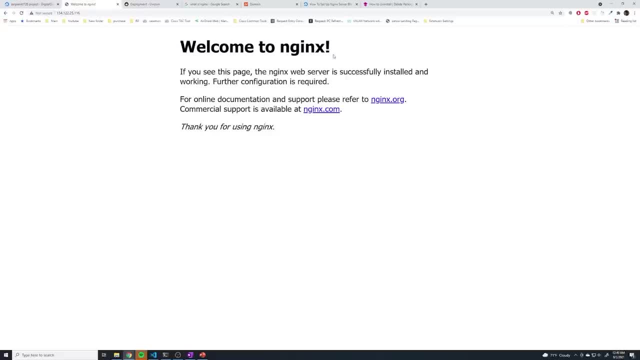 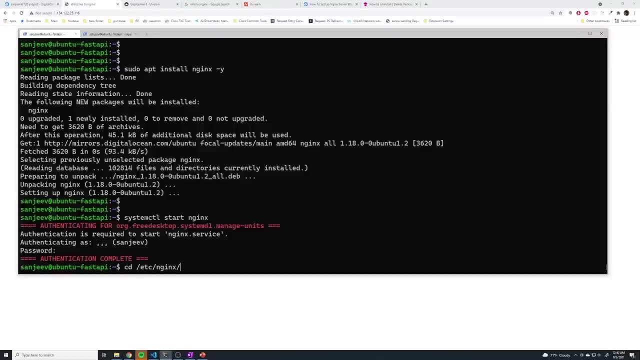 get this welcome message. So this is just the default page that NGINX loads up for you, And we're going to change this. So in NGINX, what we want to do is we want to go to slash Etsy NGINX. 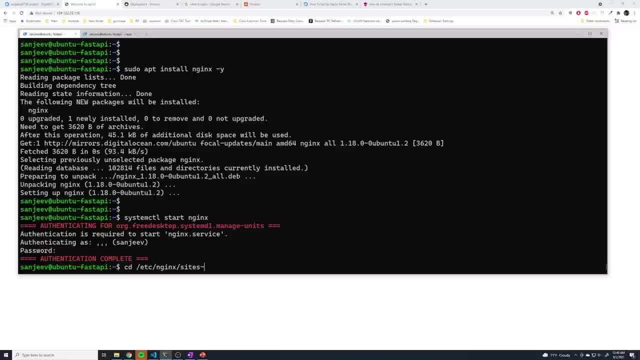 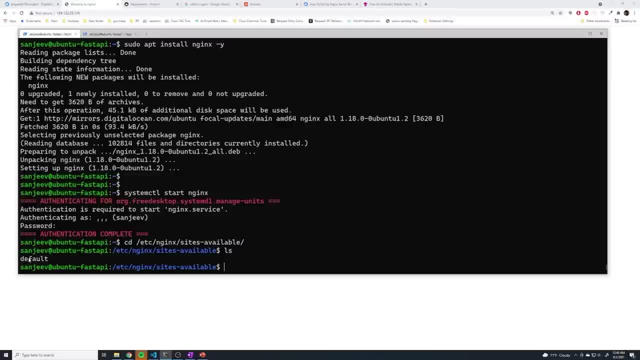 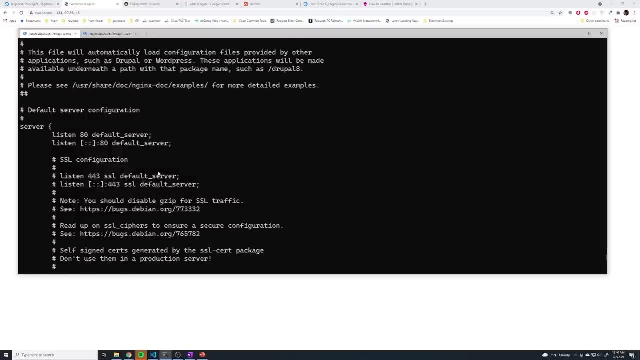 sites and then available. it's important that you do available because there's also a site enabled which is not what you want. you want available And this is default config file or technically, this is a server block And if we take a look at this, you can see the default configuration In. 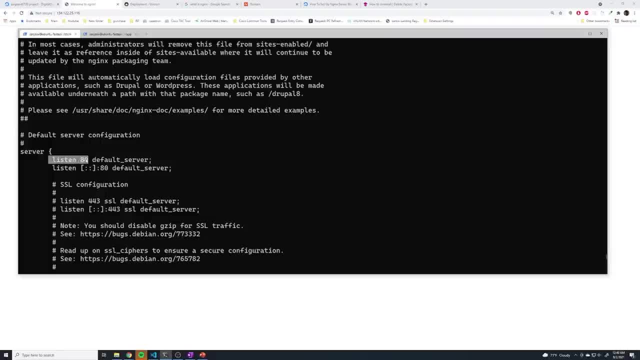 this case. just to show you what that looks like. you can see that this is handling HTTP traffic. that's why it's port 80,, it's going to listen on port 80. And this is going to act as the default server. So all requests that come here are going to land on this server block And we've got the. 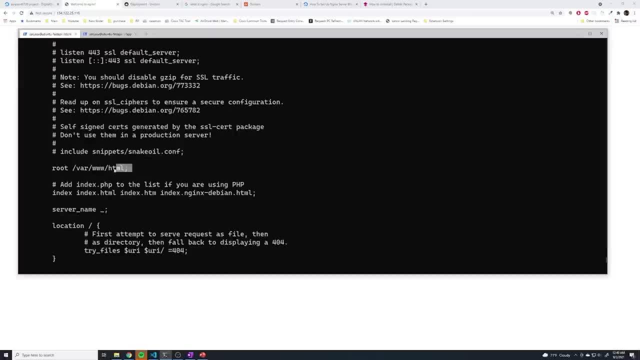 same thing for IPv6 as well, And then this is the file that you actually see. So when you navigate to this page, it's actually loading up a file that's in slash bar, slash www, slash HTML, And then the server name. So this is going to be the actual. 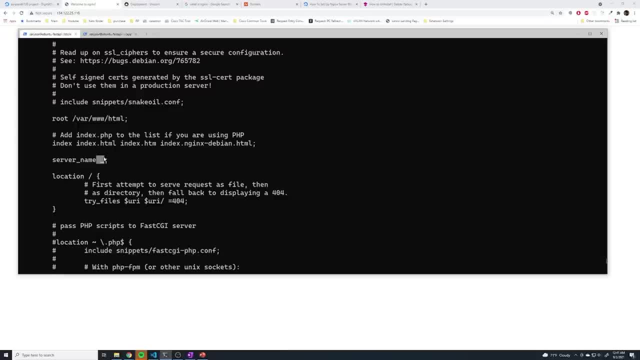 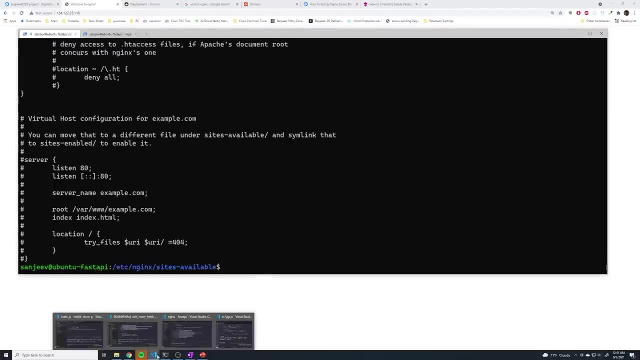 domain name that's going to handle requests, for this is basically saying everything. Everything else, don't worry too much about that. But what we're going to do is we're going to change that file a little bit, And I've provided an example file here, And so this is what an example file 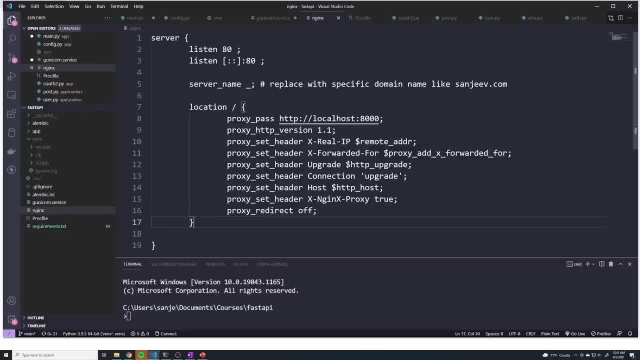 looks like we can leave pretty much everything in place. the only thing I want to change is this location block, And so this is what is going to allow nginx to act as a proxy, Specifically this line. this is the main line. you don't technically need. 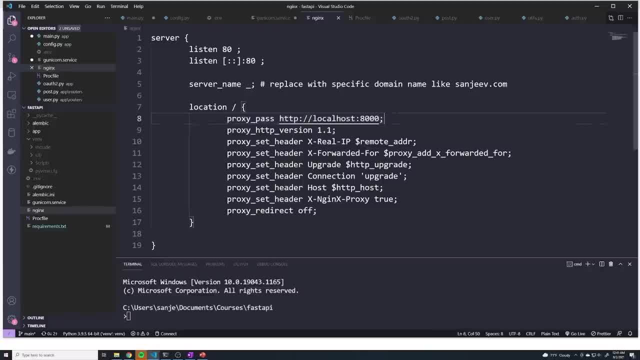 the other ones. Those are more of optimizations, But all this is saying is that any requests that match this, the, the route, path or beyond, essentially, is going to get proxied to local host port 1000, which is what g unicorns running on. So you just specify the IP address and the port. 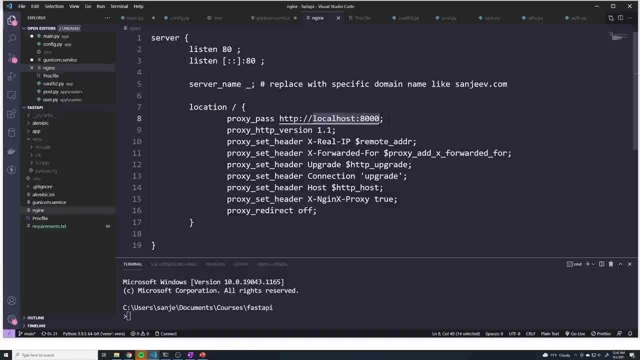 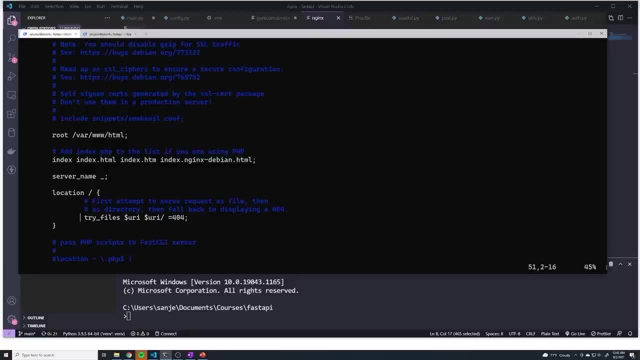 that you want to proxy traffic for, And so, since g unicorn was configured to run on port 1000, we're just going to forward it to g unicorn in this case. So I want you to just copy these lines here And we're going to go in, And I'm going to just open up that default file now And we can. 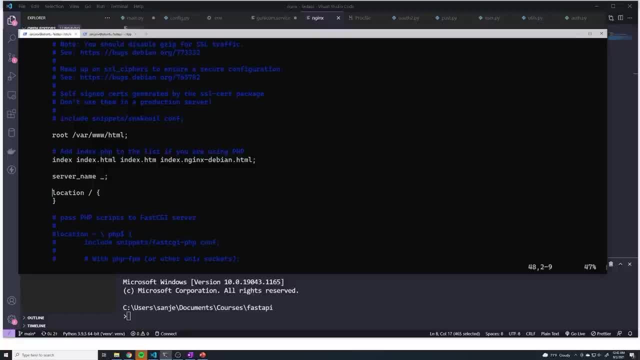 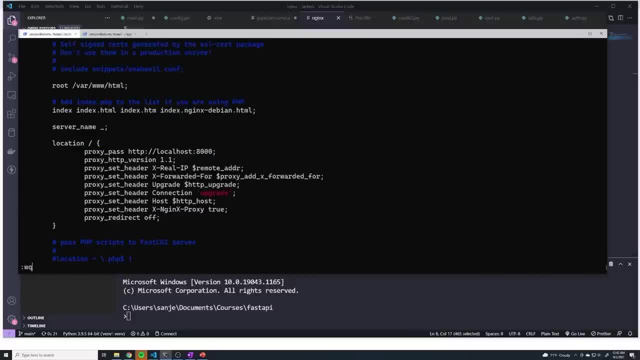 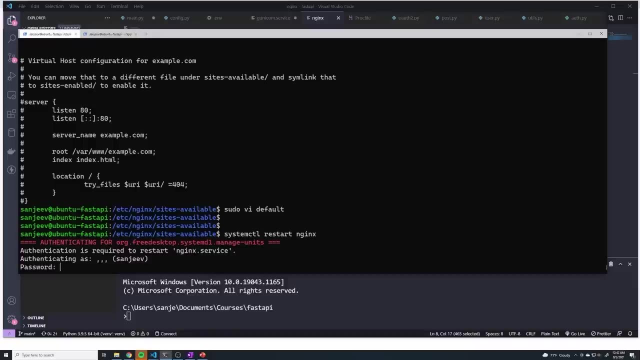 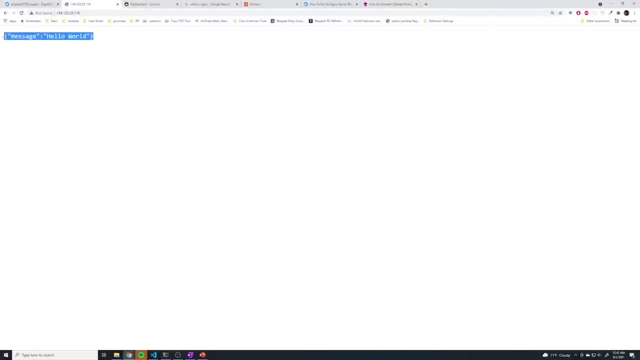 delete these three lines. I'm just going to paste that in And at that point I can save this. And then we want to do a systemctl restart nginx. So it's restarted And if I refresh this right, we can now see our API. And if I go to slash docs. 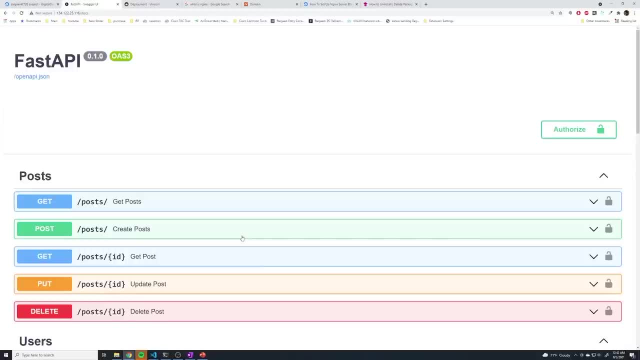 it should also work as well. So we got nginx set up And running. the last thing that we have to do regarding nginx specifically- well, it's not really nginx specific, but in general, is that right now if you take a look at it. 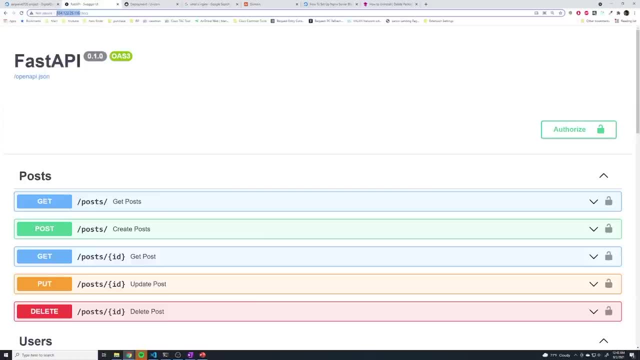 you can see, our web browser says not secure, And that's because I can actually copy this. I paste it right: we're using HTTP and not HTTPS, So we need to set this up for HTTPS. So how do we do that? Well, we're going to tackle that in the next video, But you're going to need 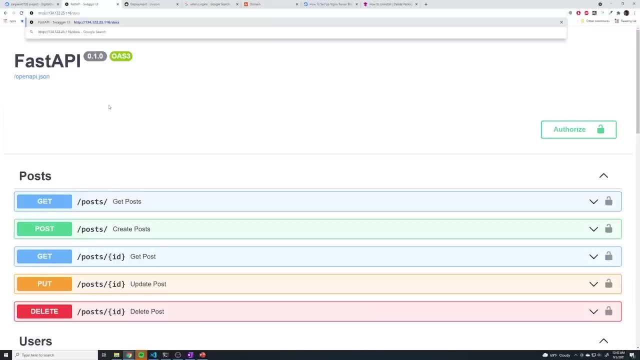 a domain name if you want this to work with HTTPS. So I'll show you guys how to kind of grab a domain name. However, if you don't have one, don't worry, you can just leave it as HTTPS for now, Or you can create a self signed certificate. whichever one works for you. 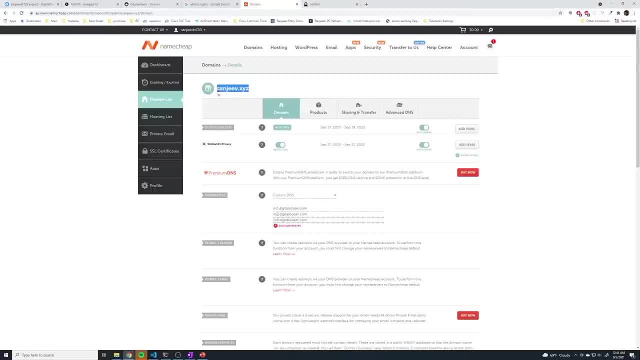 For my application, I purchased a domain name called Sanjeevxyz, So if you've ever watched any of my other videos, this is always the default domain name that I use for demonstration purposes. You can see that I actually bought a xyz because they're the cheapest, If you just want to. 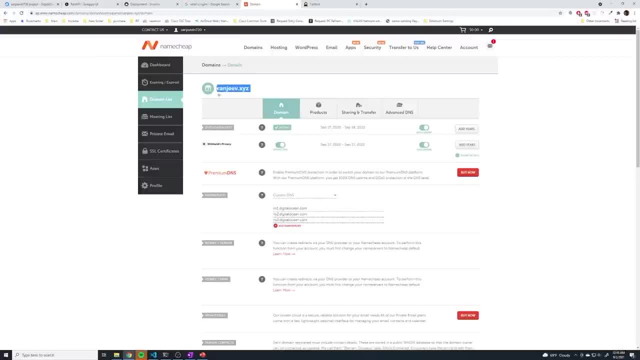 play around, just for learning purposes. get a xyz. They're usually like a dollar for like an entire year, But if you get a com it's going to be a little bit more expensive. However, depending on you, know what your domain. 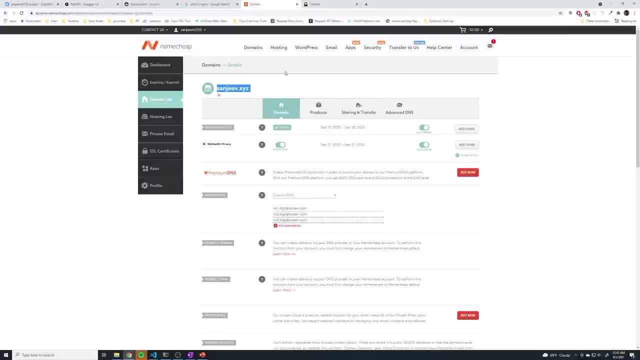 name is. it at most is still? well, not at most, but it'll. you can still find plenty at $12 per year, So it's not too bad. And I happen to purchase my domain name from namescheap, So this is my. 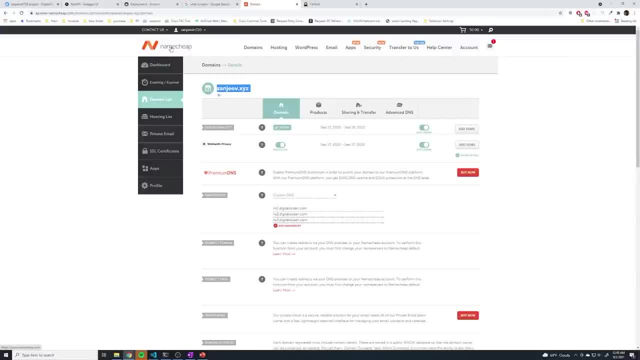 domain registrar. However, there's plenty of other options. If you want to use GoDaddy, if you want to use any of the other, any of the other websites, you can even use Amazon, if you wanted to feel free to use whichever one you want. If you want to use any of the other websites, you can even use Amazon, if you wanted to feel free to use whichever one you want. 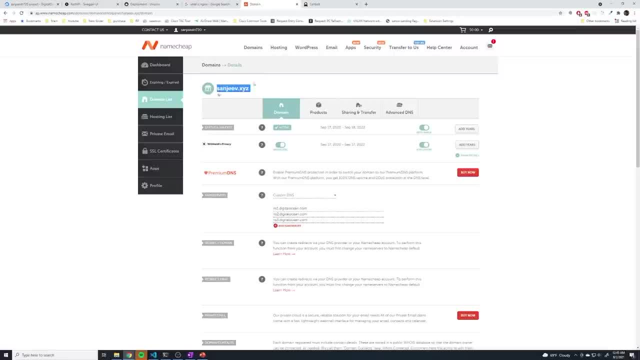 You just need to get a domain name. I'm going to be using this one moving forward, But just keep that in mind. And what we want to do is we want to set up a couple of rules And we actually have to point our domain name to DigitalOcean, And DigitalOcean has this excellent write up how to. 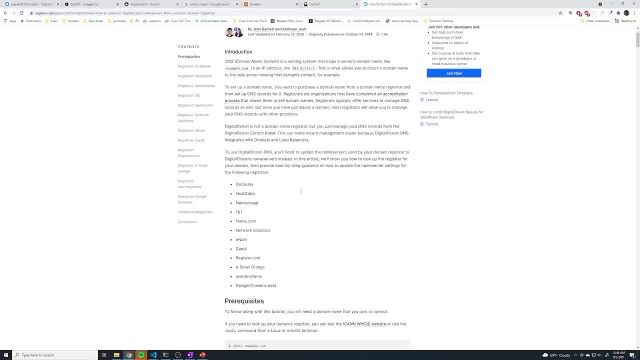 point your DigitalOcean name servers from common domain registrars And they actually show you how to do this for a lot of the main domain registrars And they have namescheap here as well. So if you get one of these, you can just follow along, But you'll see that you know any domain provider. 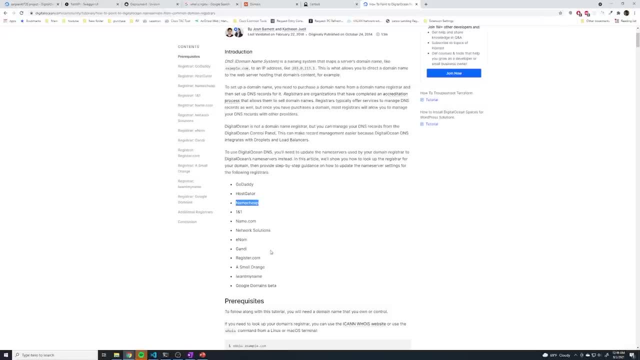 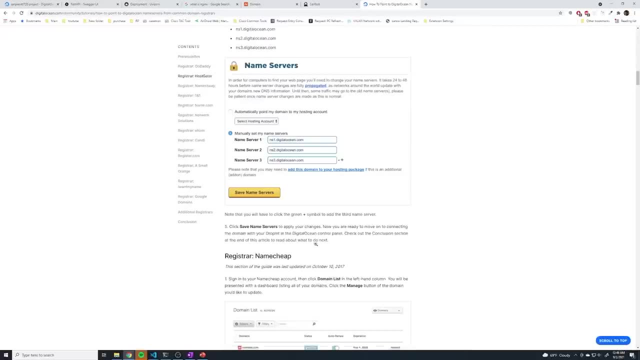 you'll be able to kind of relatively click around and just kind of navigate yourself and figure out what's the equivalent, because for the most part the UIs are all fairly similar. But if we go to down to namescheap, you can see that what we have to do is, under the name server section we have to 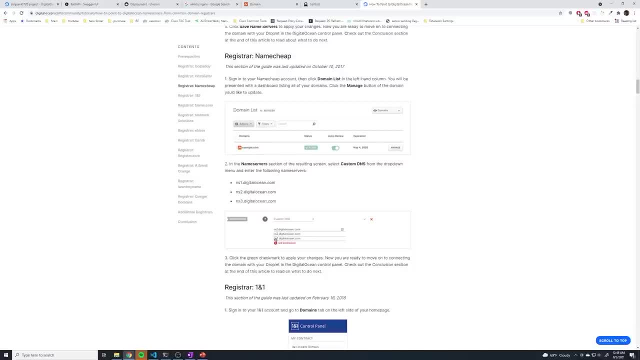 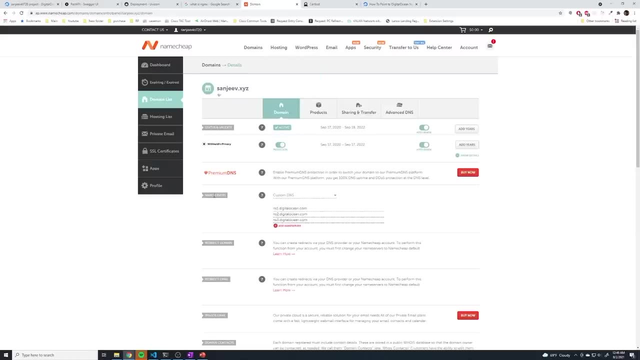 do custom DNS And then we point it to the DNS servers of DigitalOcean, So ns1.digitaloceancom, ns2,, ns3.. Let's do that, And I've actually already set that up for us, So you just go under name. 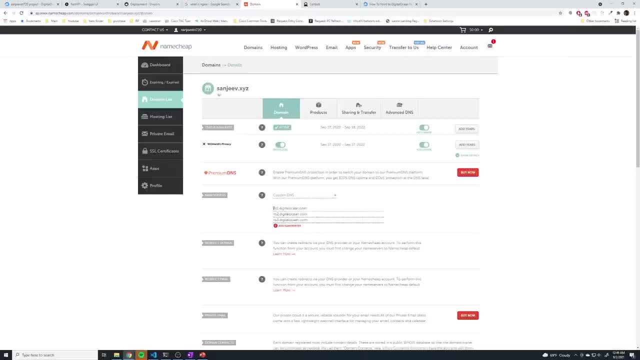 servers select custom domain, custom DNS, And then you have ns1.digitaloceancom, ns2.digitaloceancom And ns3.digitaloceancom And there'll be a little checkmark. So just check that there And at that point it's going to point everything to our DigitalOcean servers. 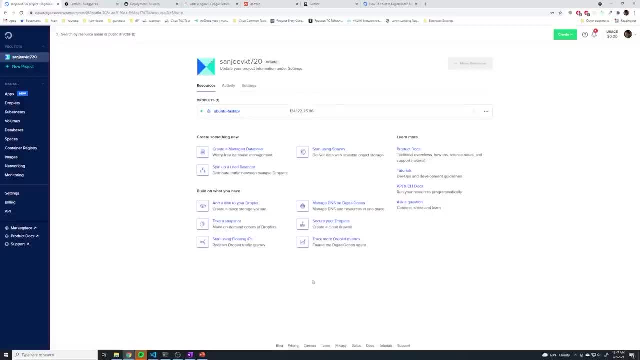 Then in DigitalOcean, if you just select your name here in your dashboard, what you want to do is you want to go to manage DNS on DigitalOcean And then here you want to enter your domain. So this is going to be sanjeevxyz. We'll add this. 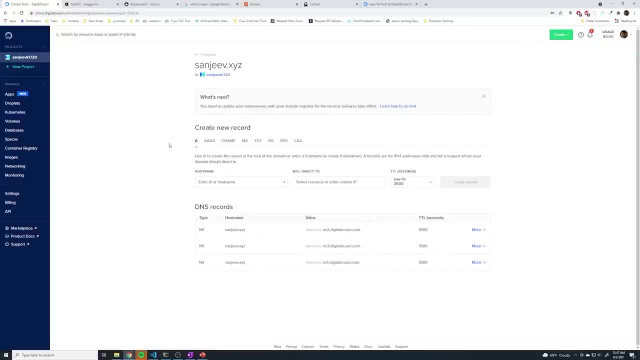 domain And the first thing that we have to do is we have to create an, A record. So this is the root of your domain. So I'm just going to say at symbol: This is going to create an, A record And we want to select the specific droplet that we created. So this one is Ubuntu. 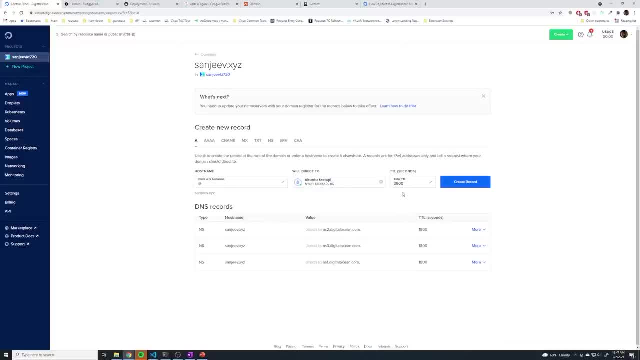 FastAPI, you should only have one. But if you have other droplets, make sure you select the right one and then select create record. And at this point if we do sanjeevxyz in our web browser, it's going. 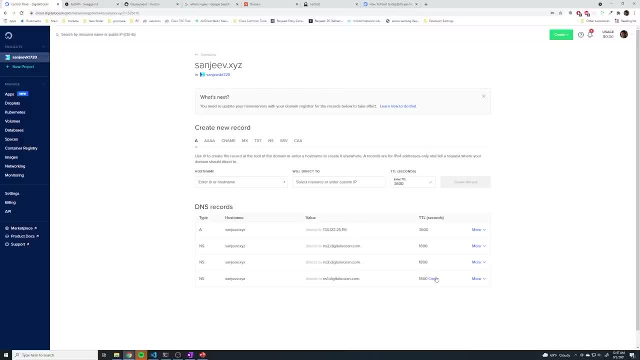 to take us to our digital domain, So I'm going to go to our digital ocean server. However, keep in mind the the changes to DNS usually take a little while to propagate, So you could potentially have to wait up to an hour or. two hours. namecheap says it could take up to a day, but it never takes a day. So if you don't see these changes immediately, just give it, you know, 1015 minutes and then you'll see that they work. But I'm going to add one more, And that's going to be for my sub domain, because I don't. 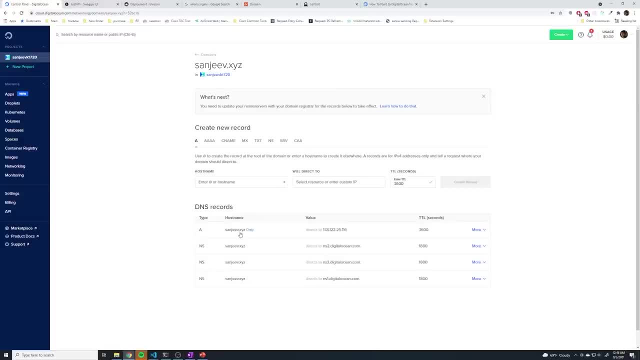 want to just do sanjeevxyz. I also want to redirect wwwsanjeevxyz to my server, So I can go to my record And I can say www, And so you can see what this is going to look like, And I'm 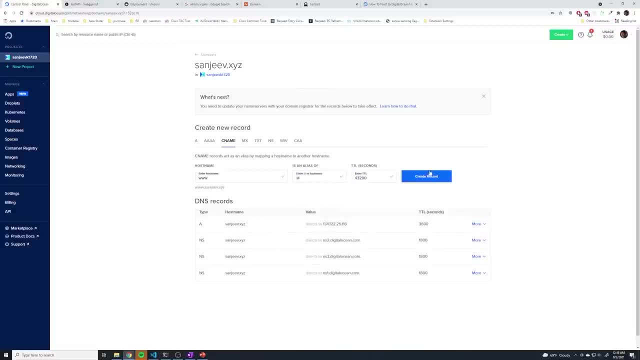 just going to say at symbol right here that's going to point it to this record. essentially, All right, And so what this is, what this is saying, is that if you send a request to sanjeevxyz, it's going to send it to the IP address of our server And then, if you send a request to the 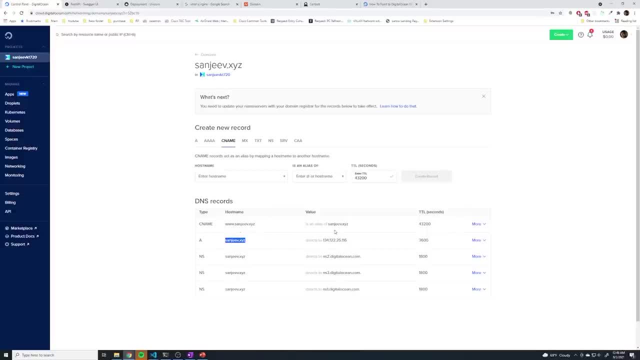 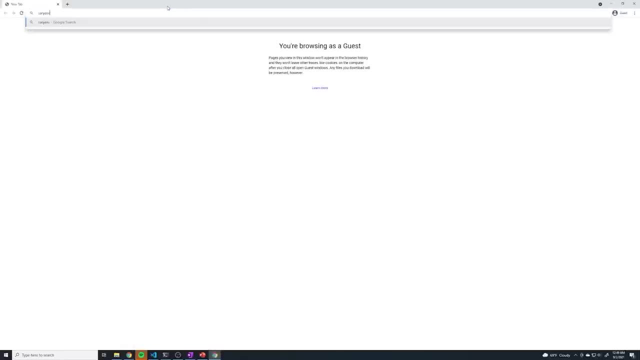 sub domain of wwwsanjeevxyz. it's going to be an alias for sanjeevxyz, So it's essentially just going to follow this. All right. So now, if I go to sanjeevxyz, you can see that we are successfully able to access our API, And if I go to slash docs. 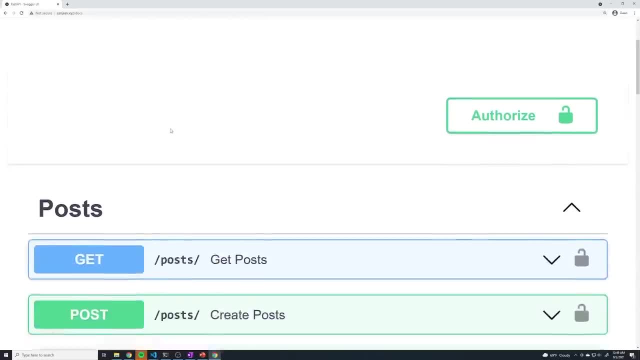 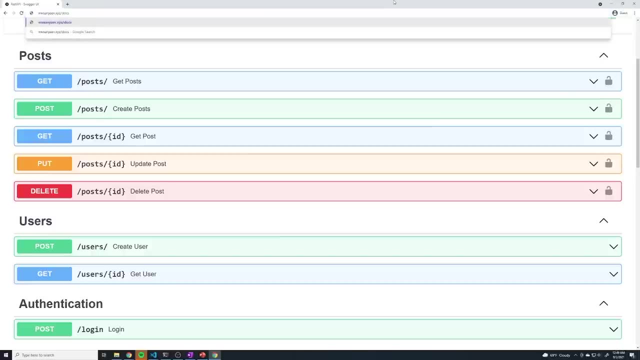 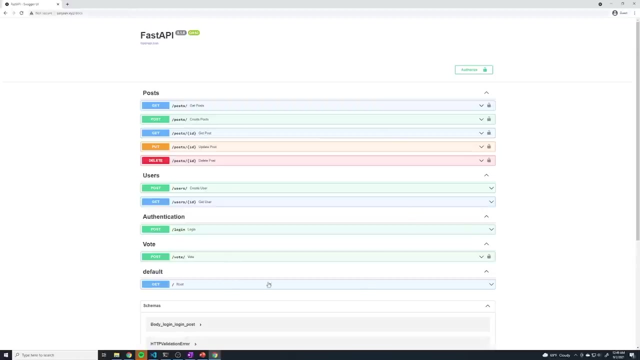 once again. this should still work as well, And that's pretty big. Let me minimize that, And if I do the same thing for my sub domain of wwwsanjeevxyz, This should also work All right. so we've got our domain setup, And once we have our domain, we can now finally set up. 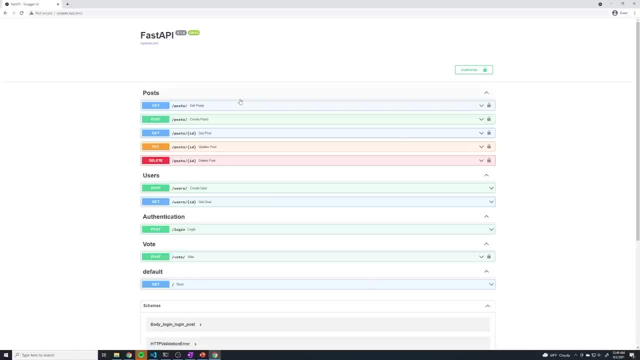 SSL so we can handle secure HTTPS traffic, because we don't want to send our application traffic over HTTP And we want that nice little lock symbol, that green lock symbol, So we'll tackle that in the next video. Okay, so it's now time to set up SSL for our application, So I want you to search. 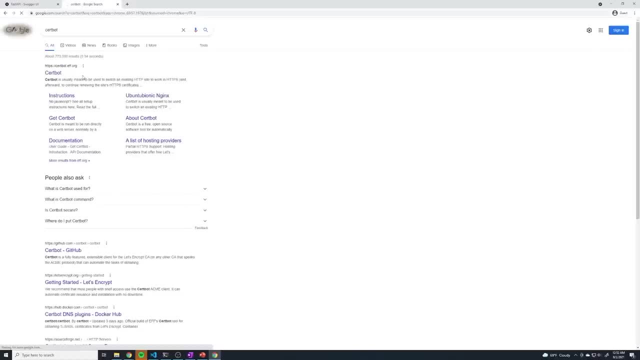 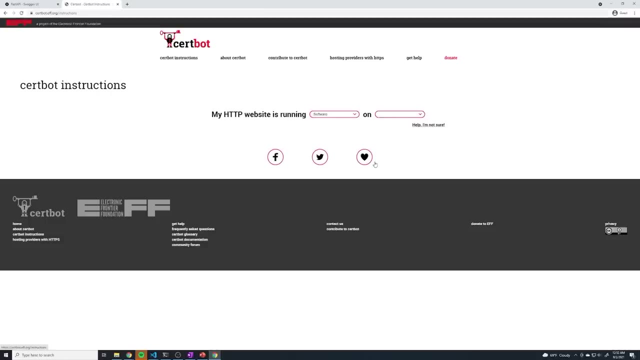 for certbot. So this is the website for Let's Encrypt, which is a free SSL service, And here they've got excellent documentation. So let's go ahead and do that. So let's go ahead and do that documentation. what we want to do is select to get certified instructions, And then we can just 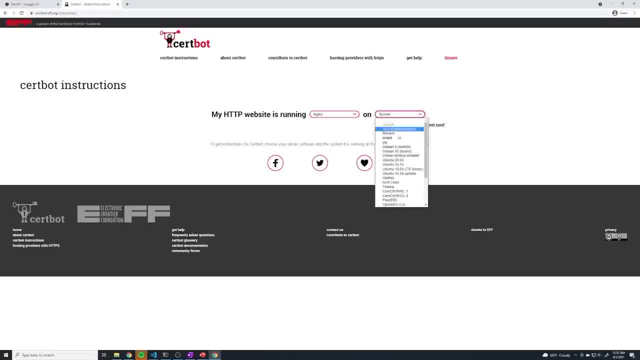 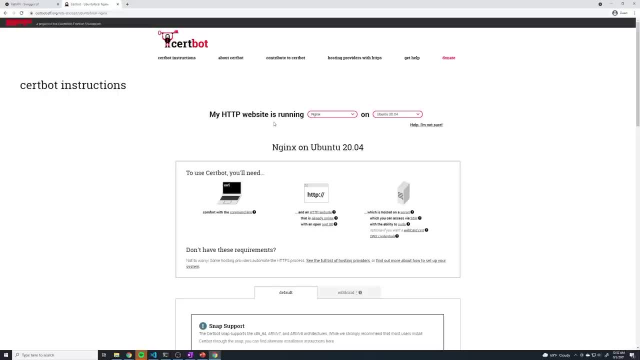 specify what software we're running. So this is for nginx And the system is going to be Ubuntu 20.0.4.. The reason it asked for this information is that it actually will automatically reconfigure nginx for you to handle HTTPS, Because normally when you want to set up HTTPS, you have to change. 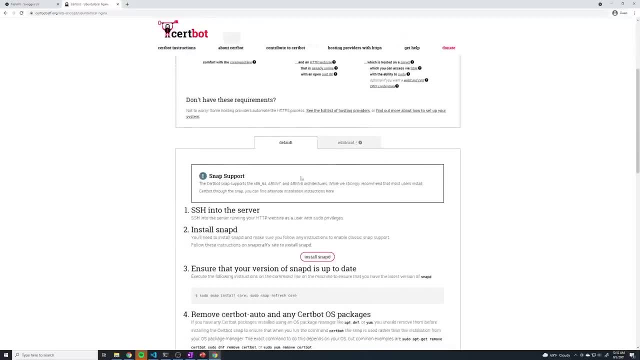 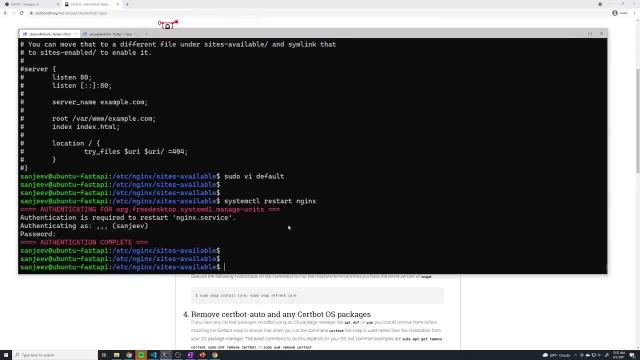 some configs in nginx and it gets a little complicated, And so the it's saying the first thing that we have to do is we have to install snapd. If you installed Ubuntu, you know from DigitalOcean- snapd should automatically be installed for you. So you. 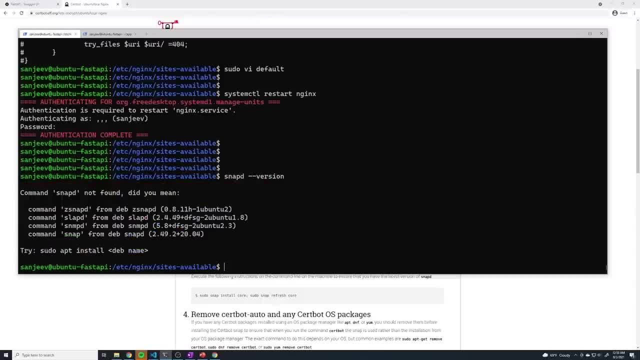 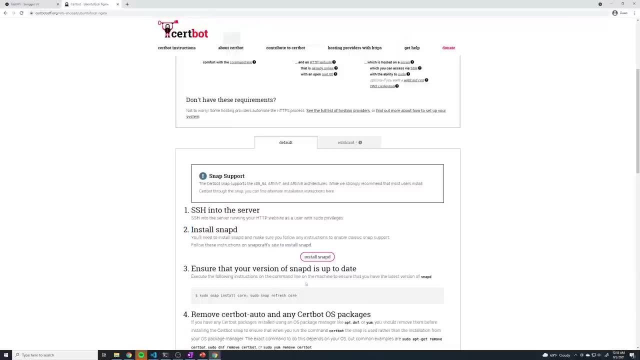 can do snapd dash dash version, I think. Or is it snap dash dash version? I think it's snap version. Yeah, Okay, so it's snap. Okay, so we've got snap installed. That's perfect, And then what we want. 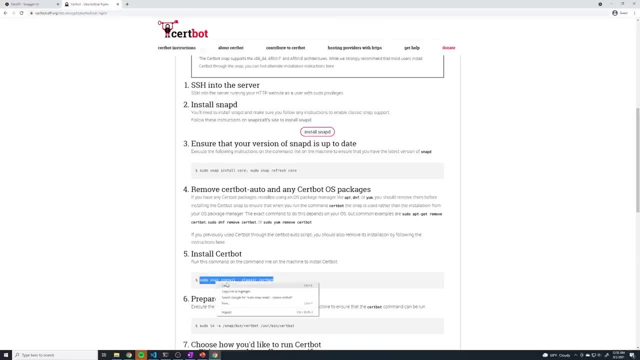 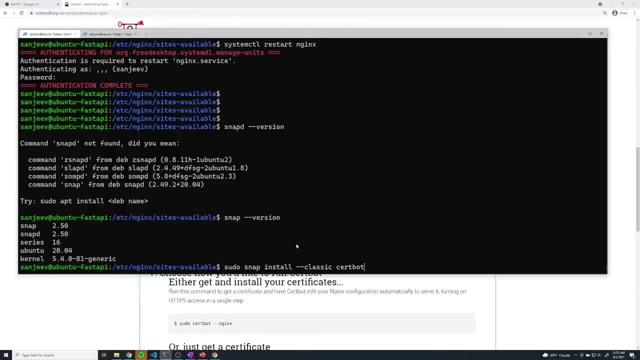 to do is we want to install with this command right here. So just copy this And we're pretty much just going to follow this website because I told, like I said, the instructions are fantastic, So we'll install certbot. All right, certbots installed, then we want to do this command. 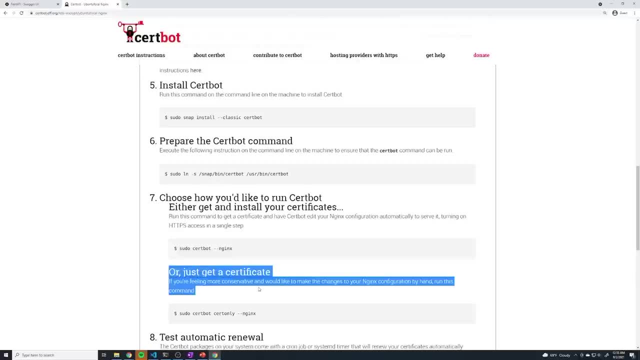 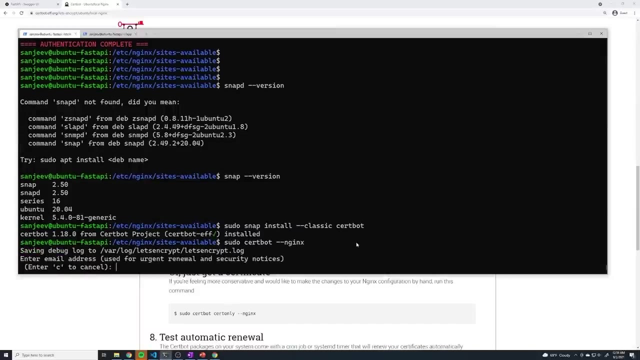 But you have two options. you can either just generate a certificate, Or you can have certbot automatically configure nginx for you. we're going to have certbot do the work for us, And so we can just paste this in, All right, and then we have to provide an email. 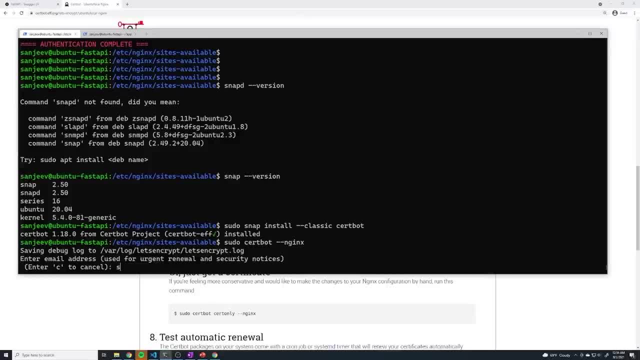 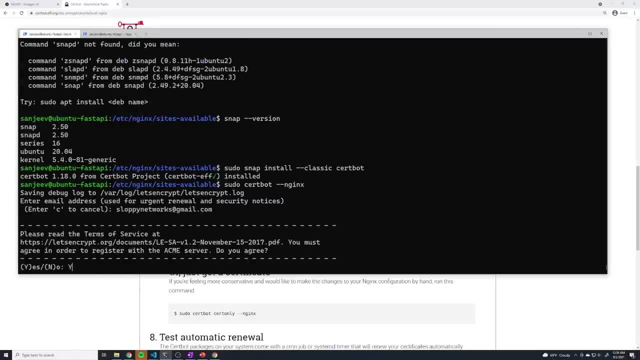 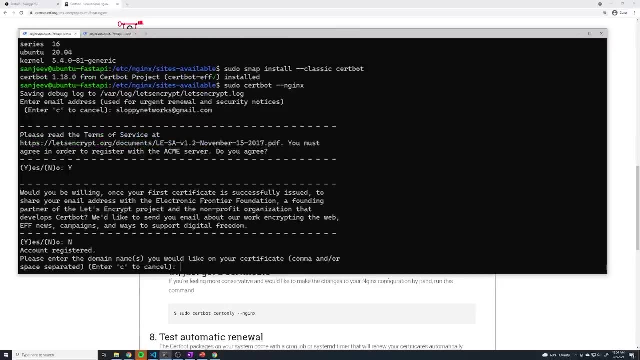 address. So this is going to be nginx, And then we're going to have certbot do the work for us. So this is going to be whatever email you want to use. And then we got to agree to the terms of service. You can do no for this one, Right? then we have to specify what domain names we want to generate a. 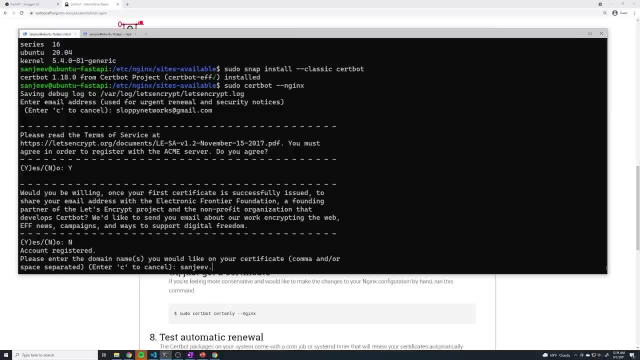 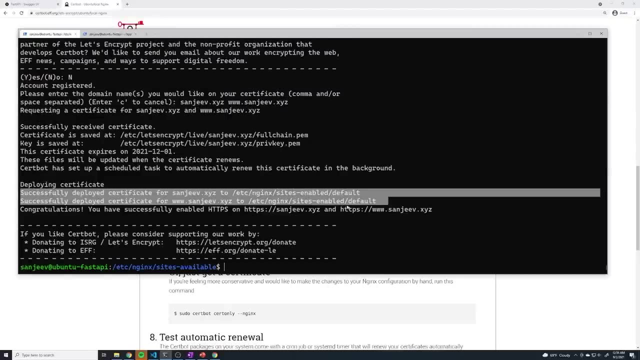 certificate for. So we want to generate a certificate for sanjeevxyz in my case and then wwwsanjeevxyz. see, All right, and it looks like it did some magic to our default config file that we were the we were originally changing. So if we actually go to the sites available folder, which we're already- 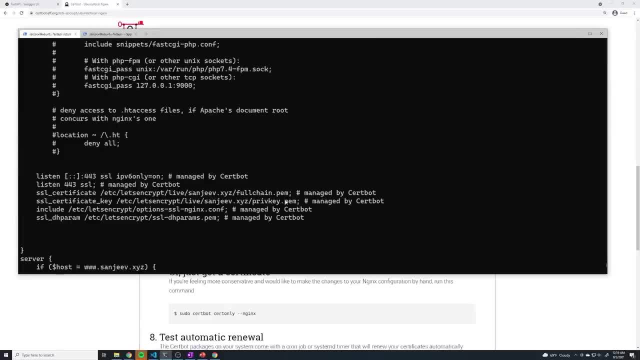 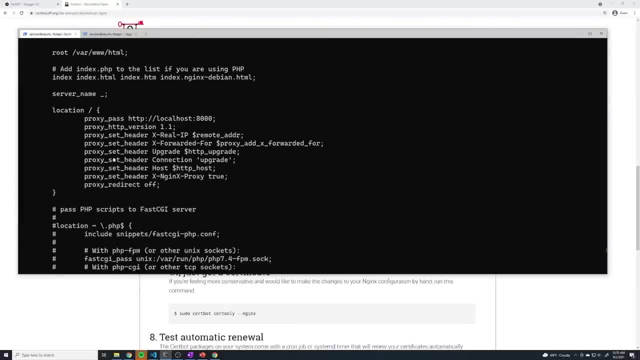 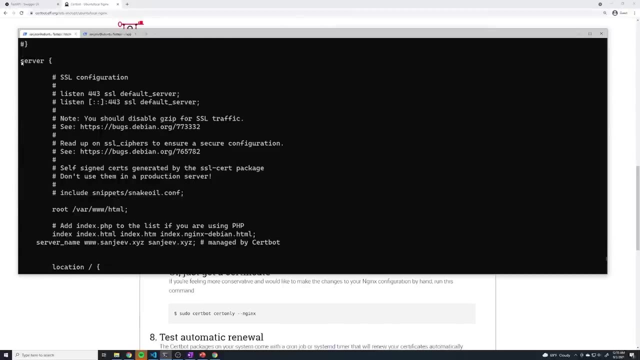 at and just do a cat default. you're going to notice some changes to this file, And that's because certbot actually made a whole bunch of changes And the main change is where. where are these changes? Not here, not here. Here we go. So this server block is for SSL configuration. 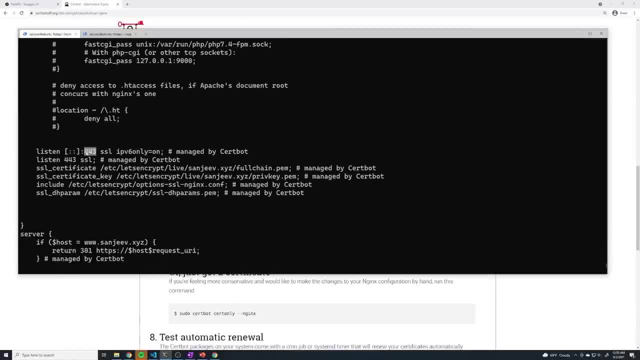 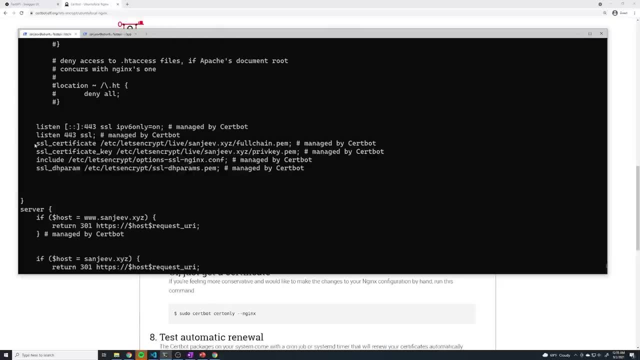 And so these are the changes they made. So we're going to listen on port 443.. So that's the default SSL or HTTPS port. That's good, And I guess that's for IPv6.. This is for IPv4.. These are going to be the two certificates that were generated, And then there's a few other. 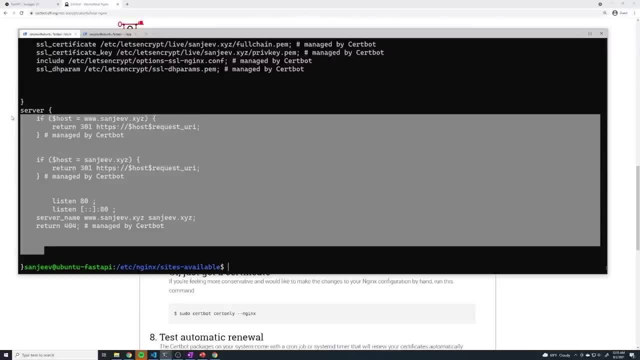 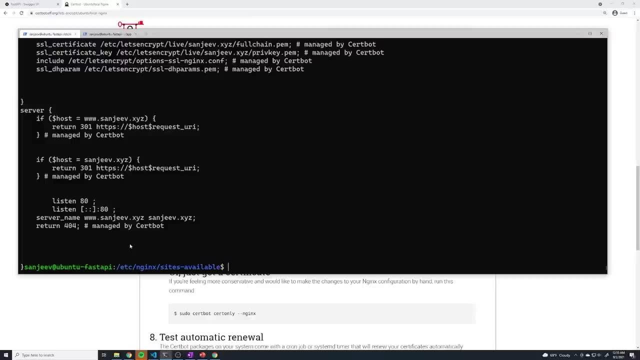 configs that it added, And we also have this server block right here, which is going to actually redirect HTTP request to HTTPS, So we can never even use HTTP anymore. it's going to ensure that our clients always use HTTPS and it'll redirect them to HTTPS, And you can see. 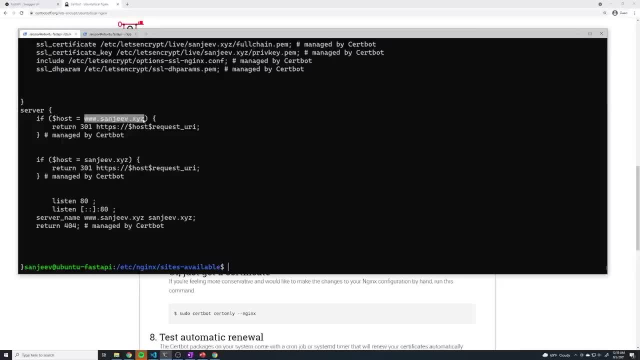 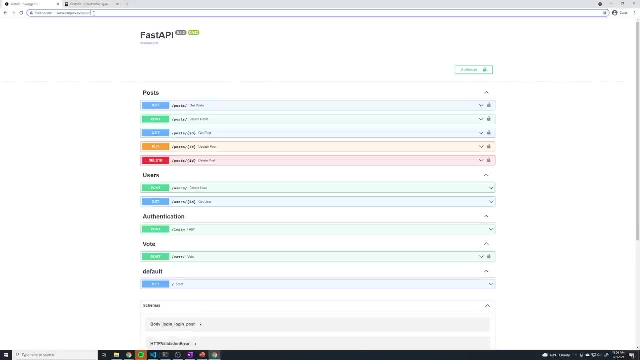 that right here. you know, if host equals wwwsangivexyz, we want to send a 301 redirect to HTTPS and then host request right here, And we're doing the same thing for just the sangeevexyz, And so that's all done by cert bot. And so now, if I go here and I do, 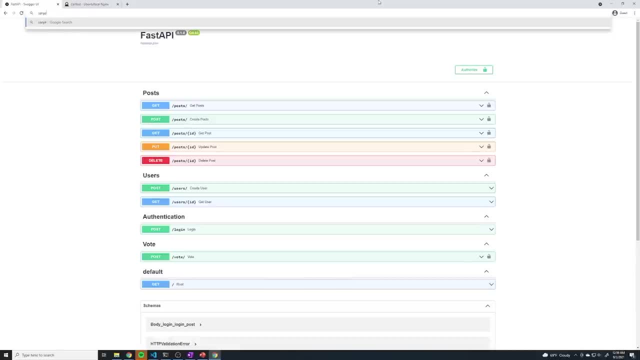 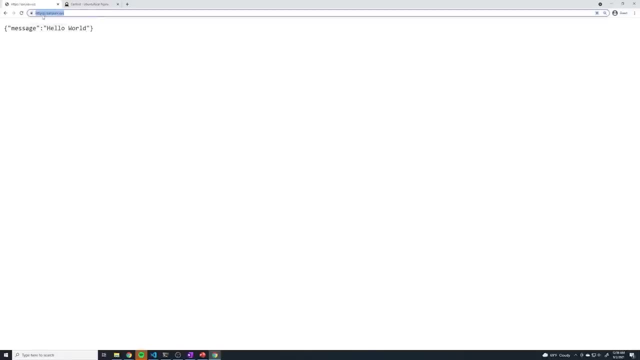 sangeevexyz. take a look at this. we get the little green lock. that means connection secure. that means we're using HTTPS And you can see the HTTPS here. And if I hard code it to be HTTP, look at that. it still has the lock because it redirected to HTTPS. 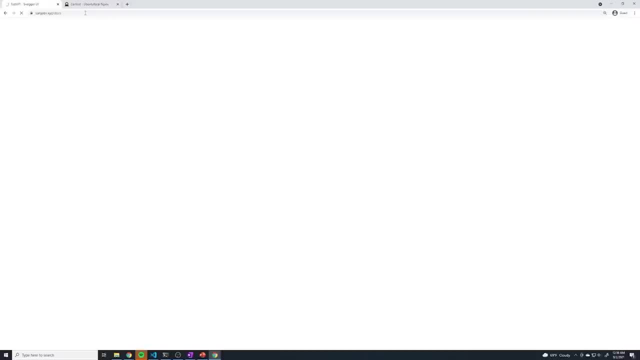 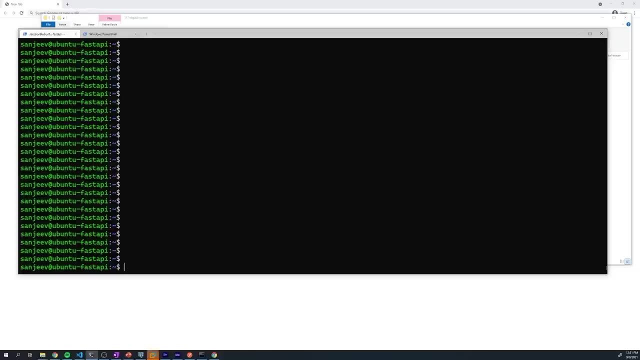 And let's just make sure that the docs work now, And it looks like the doc still works. So we now have HTTPS set up on our Nginx server And, just like we did with our service, we want to make sure that Nginx has been set up to. 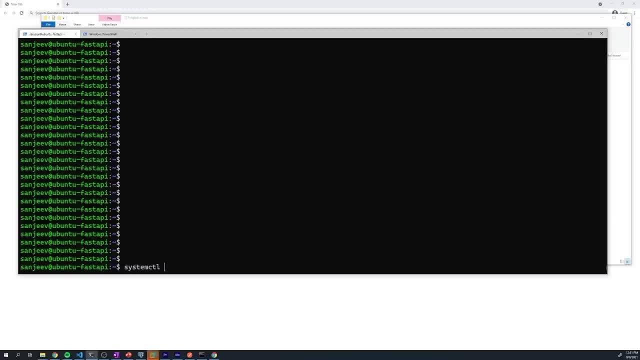 automatically start upon a reboot. So we could do a system CTL status Nginx, And let's just quickly verify if it's, if it has been set up to do so- And I can see that on mine it's set up to be enabled, So it will automatically start upon reboot, which is what we want. 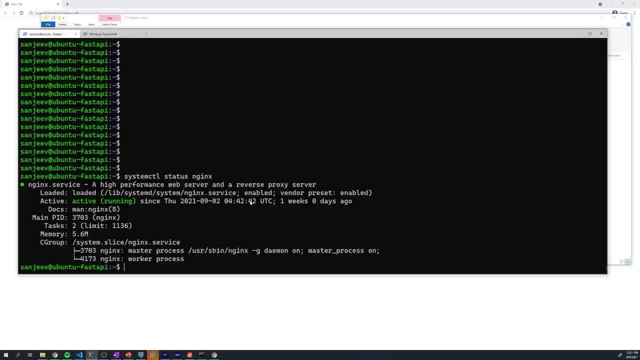 And I think this is the default configuration when you install and set up Nginx. However, if you see disabled here, just go ahead and do a system CTL enable Nginx And that's going to make sure that it will be moved to an enabled state, So it'll get started upon a reboot. 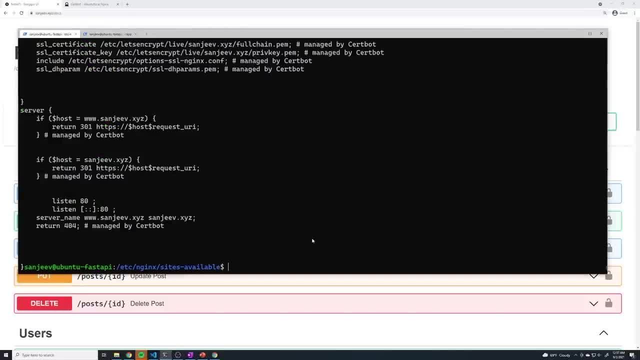 The last thing that we need to do to complete our deployment process is set up a firewall on our machine, And the reason we want to set up a firewall is just for basic security purposes. we want to make sure that we only open up ports that we're going to be using. 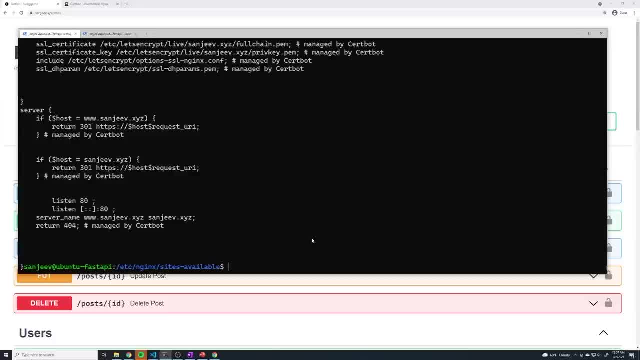 Because right now you can access this box on any port And we want to make sure that we really harden our system so that only the traffic that should be sent to this box is allowed to this box. we don't want people trying to connect to different services on our machine that they shouldn't be. 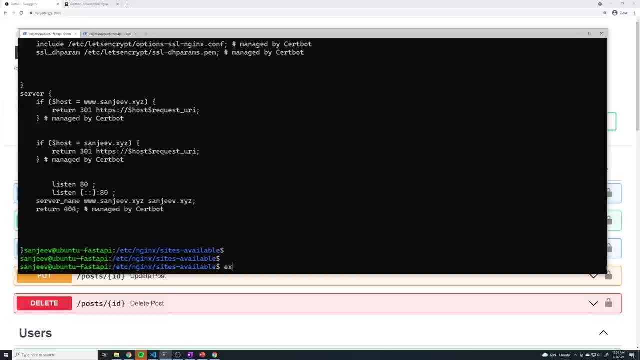 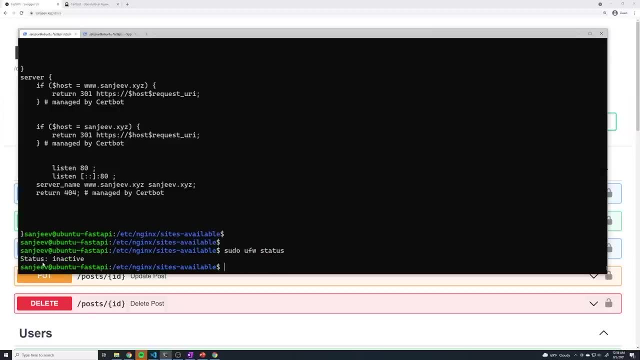 So we're going to be using a, the built in firewall called a UFW, And if we do a pseudo UFW status, UFW is the firewall And so you can see, right now it's an active and that's perfect And what we've. 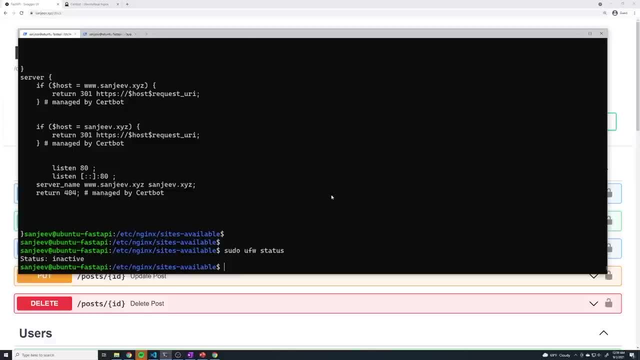 to do is we have to set up a whole bunch of rules And we have to tell the firewall what kind of traffic should we allow to our machine. And we can run sudo, ufw allow, and then we can specify, you know what specific port we want to allow traffic on, what specific IP addresses should. 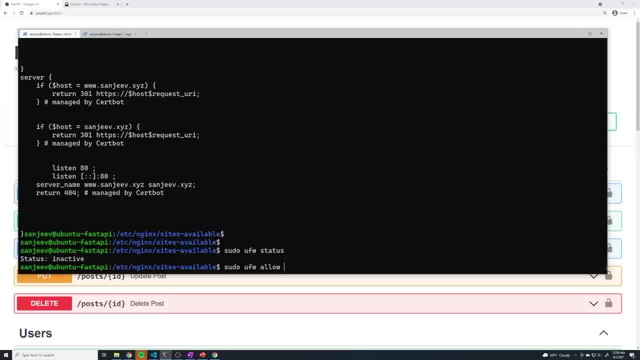 we should be able to talk to. So, since this is a public API, we want to make sure that, technically, anyone can access our server from HTTP and HTTPS. So we're going to do allow HTTP, so that's going to allow HTTP traffic And you can see it created an IP v4 and an IP v6 rule. 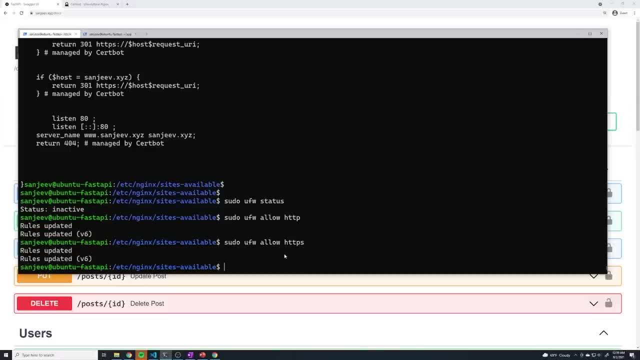 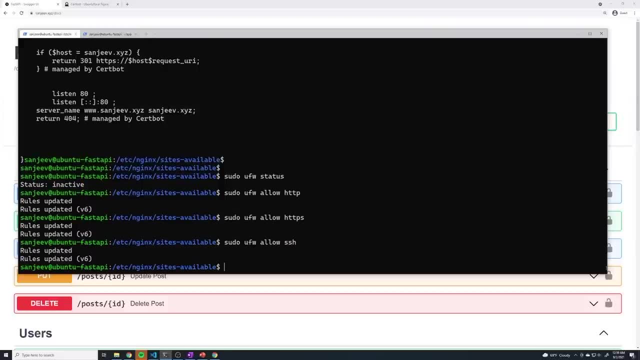 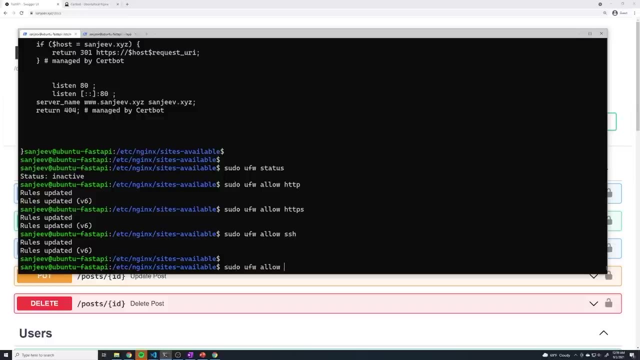 we want to allow HTTPS traffic And keep in mind, we have to SSH to our machine so we can access it. So we have to allow SSH as well And if you wanted to, you could also allow 5432.. So that's going to be to allow Postgres traffic. Now, the way we've 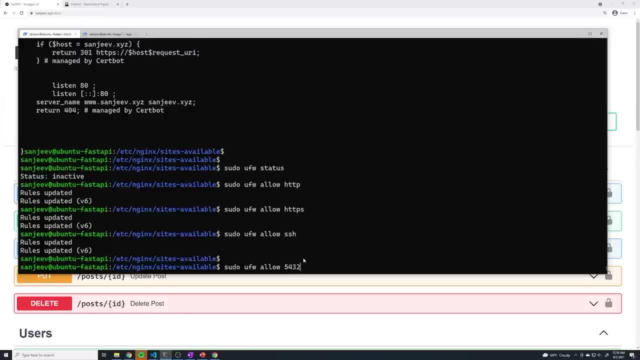 set things up. you don't need to actually allow this port Because technically, our app right, our fast API- is running on the local machine. So it's not going to be hindered by this firewall. So it can access the database because it's running on the local machine. So if you wanted to make 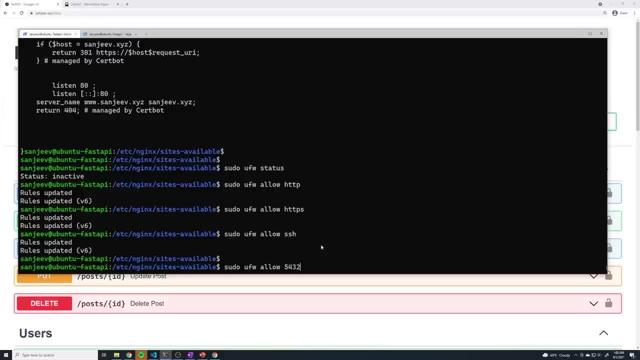 it so that no one from the outside world can directly access your database. you would not want to allow this, And that's what a lot of people do, because it can be a little risky opening up your database port, because then people can potentially access your database. So it's up. 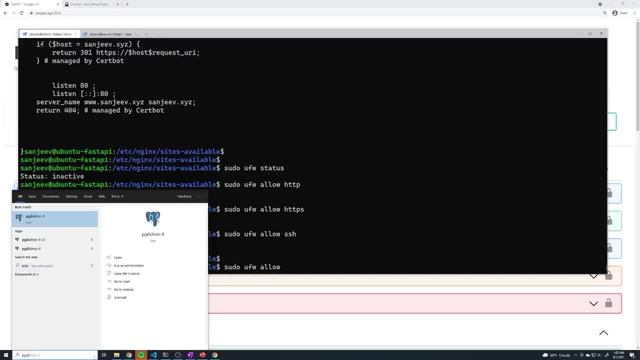 to you. However, if you want to be able to access your database, you can do that, But if you want to be able to, you know, go to PG admin. And if you want to be able to connect to your box remotely, 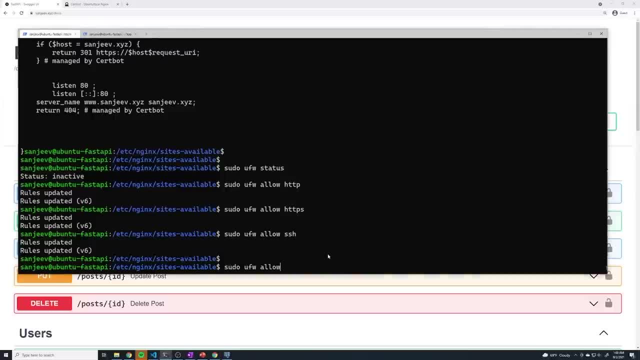 then you're going to have to allow 5432.. So it's just up to you, it's your preference, do whatever you want to do. I'm going to allow this just for demonstration purposes, So I can show you that, hey, when you allow 5432, we can connect remotely. So I'll add that rule. 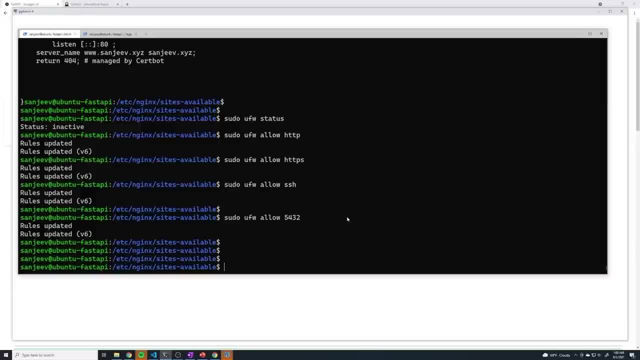 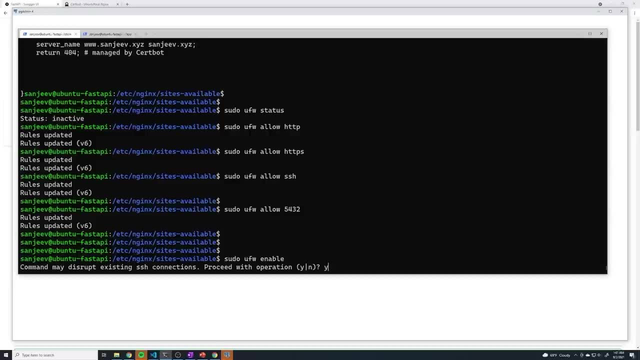 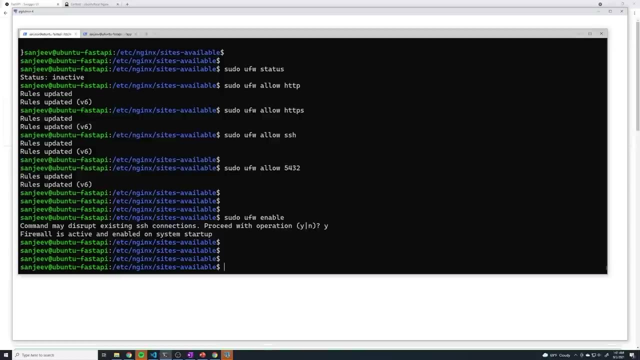 And then, finally, we have to start our firewall. We do sudo ufw enable And it's just going to tell us that we could potentially lose connection because we're starting up a firewall. that's fine And we've started up a firewall. If I do a sudo ufw status. 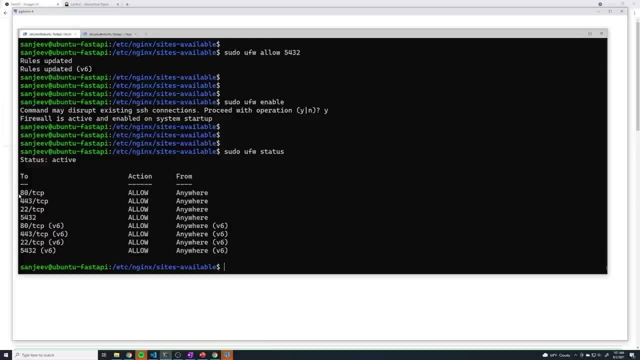 you can see that it's active And you can see all the rules that it's put in place. So it's saying we allow port 80 traffic from anywhere, we're going to allow that, port 443, we're going to allow from anywhere, And same thing with SSH and 5432.. And all of the IPv6 rules as well. 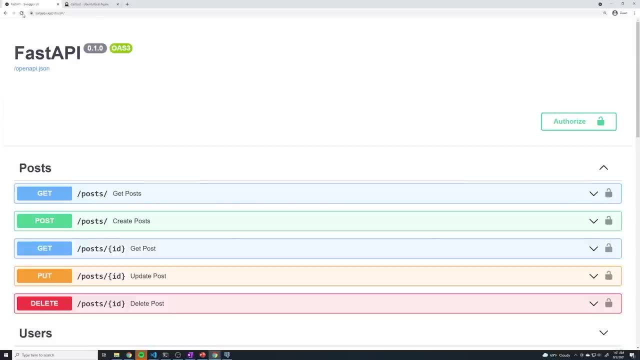 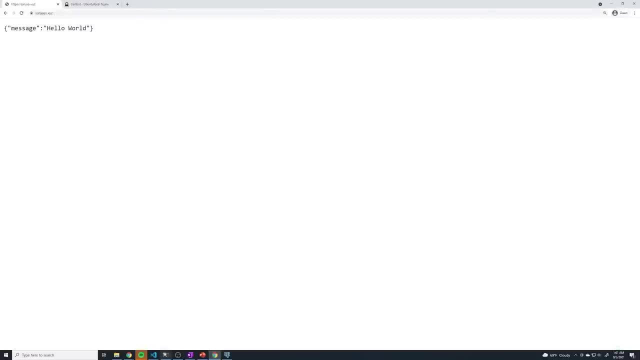 And then everything else is dropped and blocked And let's just double check that we can access the docs- And it looks like we can, and just to make sure it's not cached or something like that Still works. And now we've got our firewall. 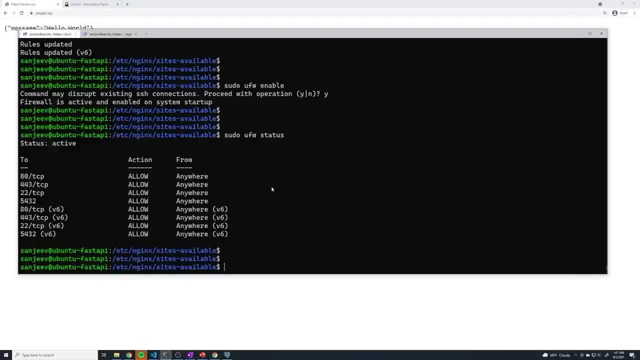 And the firewall will start up automatically, So you don't actually have to configure anything else. If you do want to delete a rule, you can do sudo, ufw- delete, allow and then whatever rule, so you can do HTTP or you can do 543 to whichever one you want to delete. 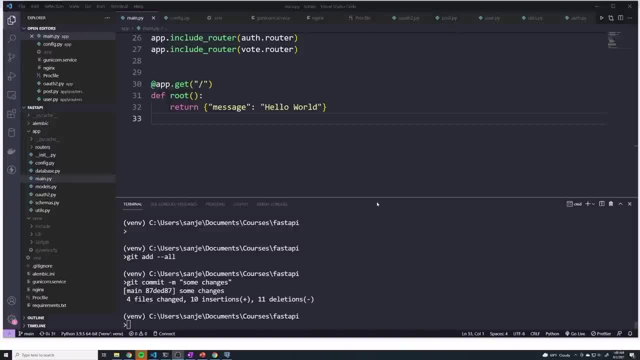 But now that we have our application deployed, one of the common things that you're going to have to do is make changes to your application and then push out those changes. So I'm going to show you guys how we can do this in a manual process. Ultimately, if you're developing an application, 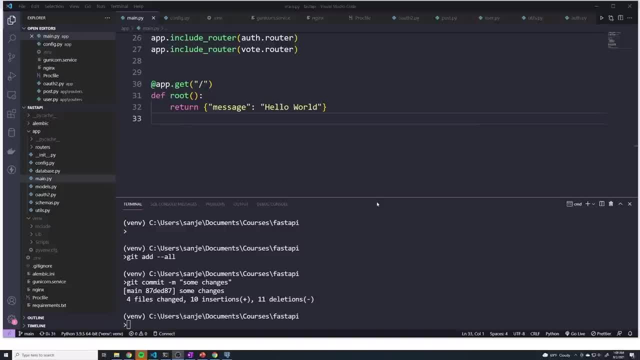 it's best to set up a very efficient CI CD pipeline, But that's a little outside of the scope of this course. So I'm going to just show you how to do this manually, And you'll see that it only requires a couple of commands. So go ahead and make your changes. you know whatever code. 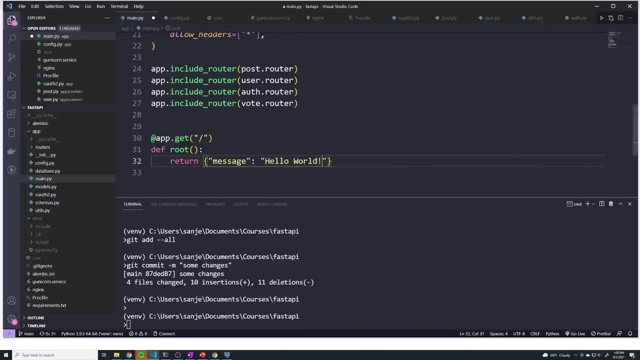 changes. So I'm going to say Hello world, couple of exclamation points, All right, we'll save that And we're going to do is. we're going to do a git add dash dash all again. And we're going to do a git commit dash m. give it some meaningful message. changed the world. 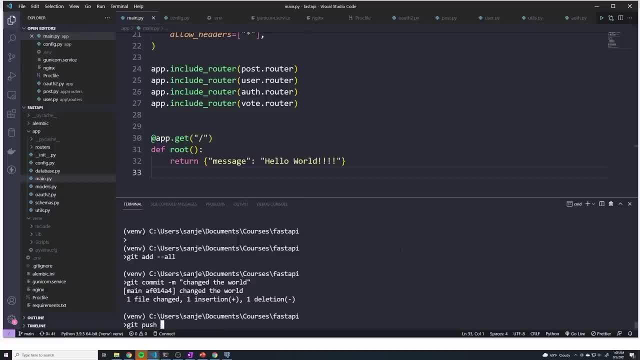 All right, and then we're going to do a git push. And before we do that, if you type in, yeah, just do a git push, Then we provide origin, which is the name of our remote, And then branch that we're on, So we can say main And that's going to push it up to our GitHub repository. 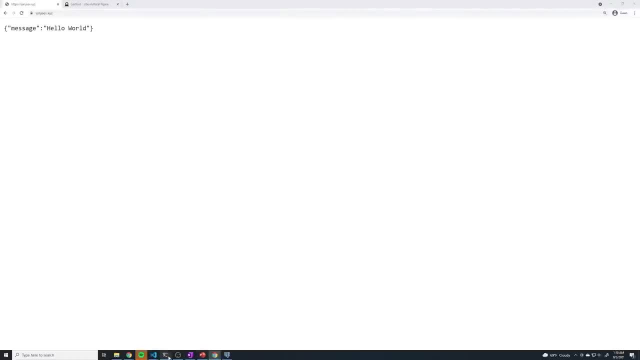 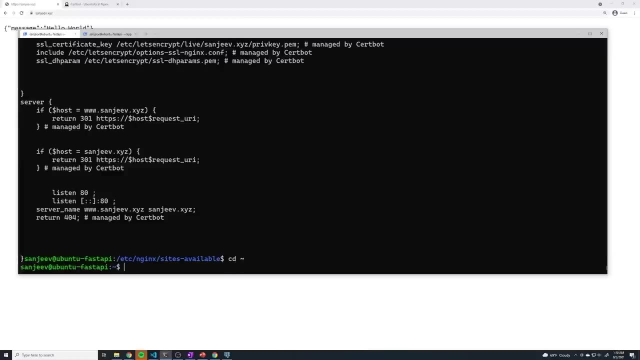 And at that point, once it's there, you can just quickly verify if you want, but I'm going to assume that it's there. And then what we're going to do is we're going to go into our application folder, which is in our home directory. then we go into apps and then source, And then here: 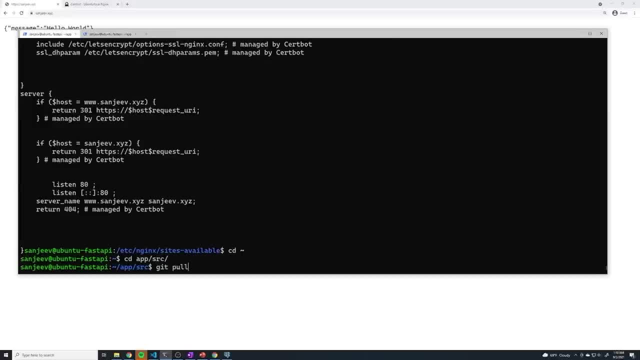 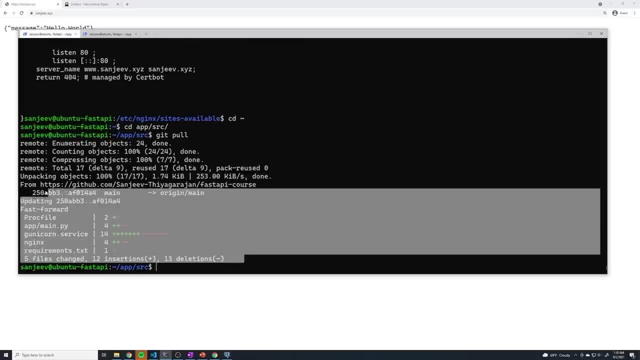 we're just going to do a git pull. So it's going to pull all the changes that were made. So it's it's going to grab the latest changes and we'll all right. so we've pulled out all of our code now and keep in mind, you know, if you had changed the requirementstxt file. 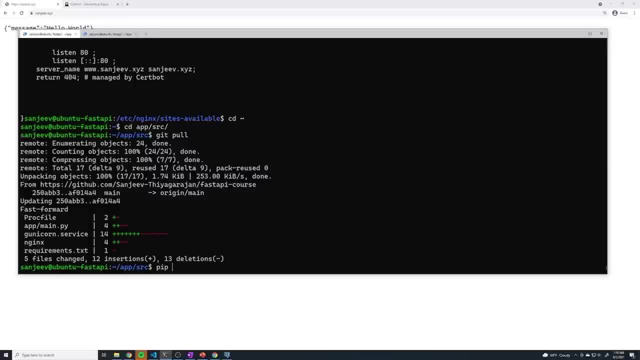 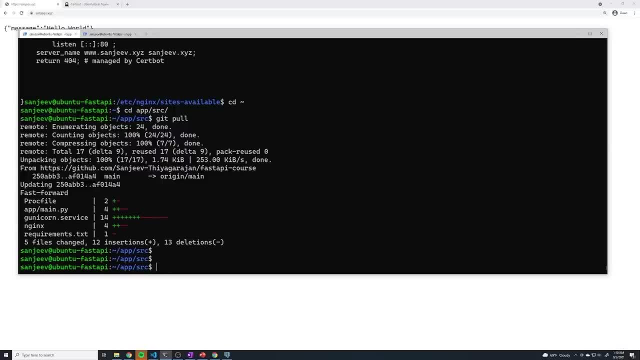 then you definitely want to do a pip install. uh, you know pip install, dash r requirementstxt if you did. but we didn't change any of that, so we don't need to do that. uh, and what we can do now is: we can we have to restart our application, because if i just refresh this, you can see: 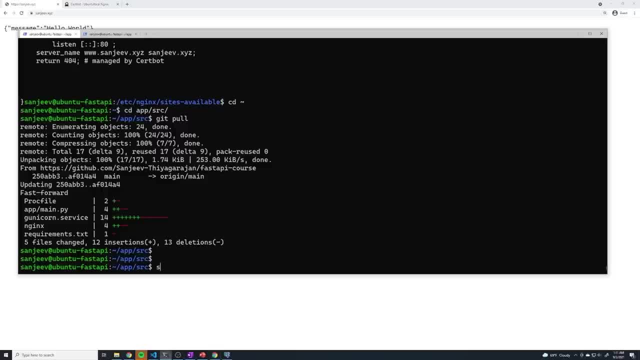 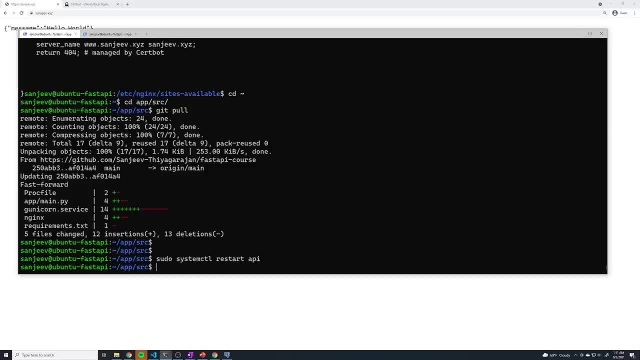 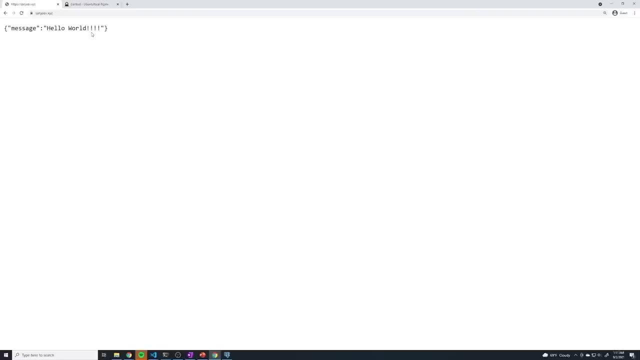 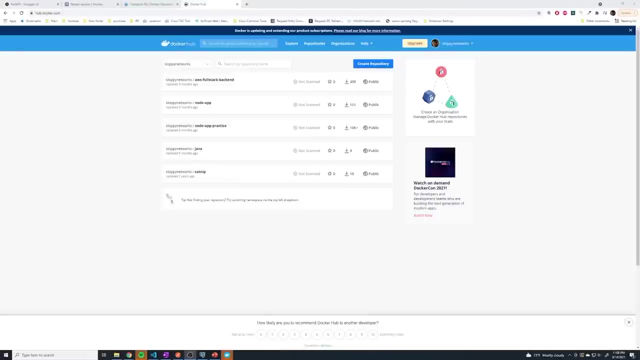 nothing's changed. there's no exclamation points. so we'll do a system: sudo system ctl, restart api battle and let's try this out now. and we've got all of the exclamation points now. so that's how you push out changes through a manual process. but, like i said, it's best to set up a cicd pipeline in this section. we're going. 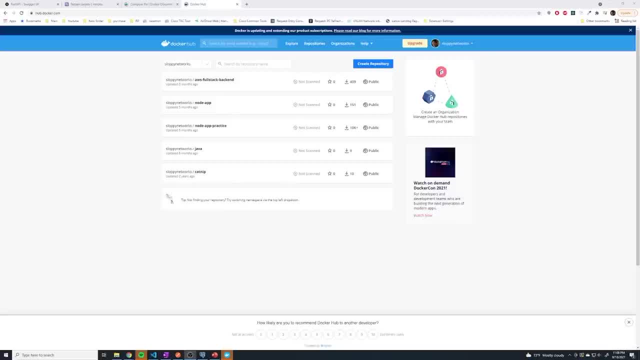 to focus on the program, focus on Docker rising our application. I originally wasn't going to do anything on Docker, but I figured I would just make a quick video just to show you guys how we can quickly set up our fast API environment within a Docker based environment. And I'll also 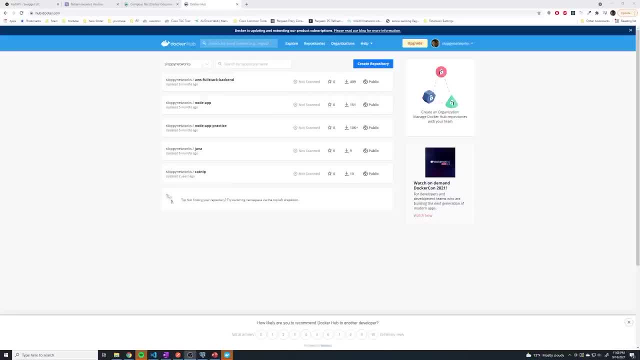 show you guys how to set up a Postgres database within Docker. This is going to be a fairly quick run through of Docker. I'm going to assume that you guys have a basic understanding of Docker. I'm going to assume that you already have Docker installed on your machine. So 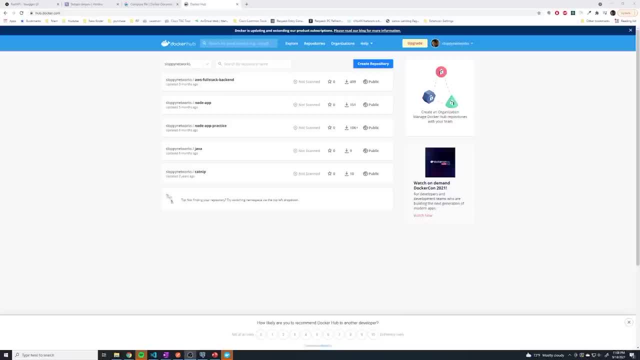 we're going to get right to it and get started on setting up our fast API within Docker. So I had Docker hub open, which is, just you know, a public repository of different images that we have access to. you can create an account if you want to. you don't have to. 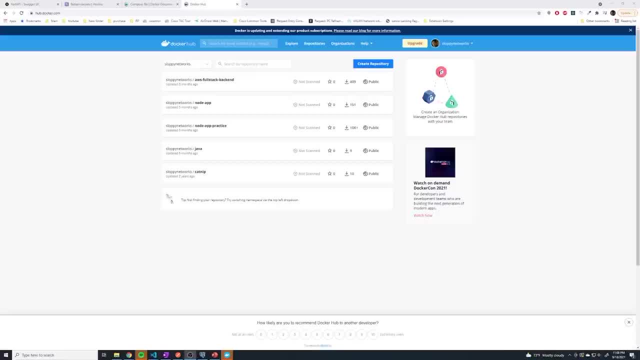 create one at this stage. the only time we'll need to create an account for this course is if you want to push an image up to a- you know- a repository hosted on Docker hub. If you don't want to do that, then you don't need to go ahead and create an account. But 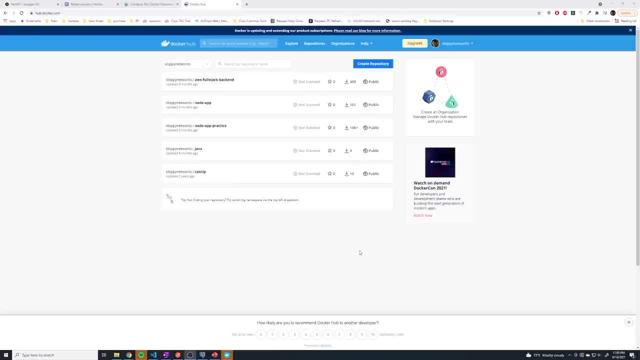 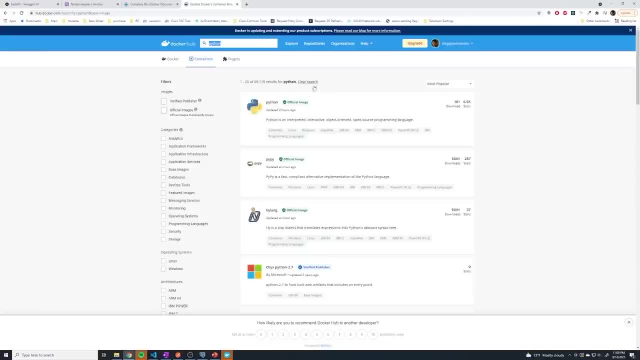 what we want to do is we want to figure out a image that we're going to use for our fast API, a Docker container, And so just go ahead and search for Python, And what we're going to do is we're going to use the official Python image. So select the official Python image And you'll. 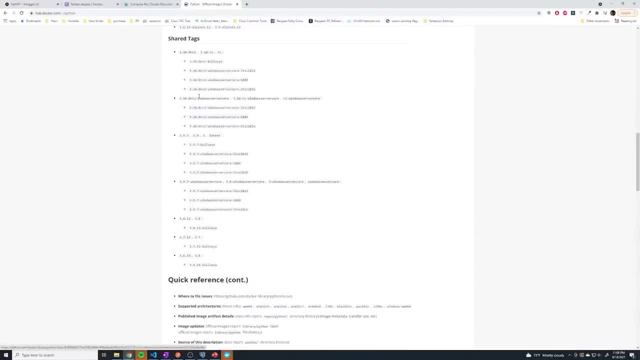 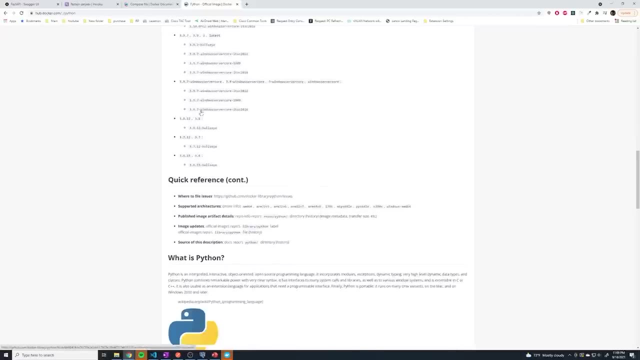 see that there's a couple of different options, So you can scroll down. you can see the different versions of Python, And we're actually going to use version 3.9, dot seven in this case. But you can see that with the default Python image we have all of the different versions. 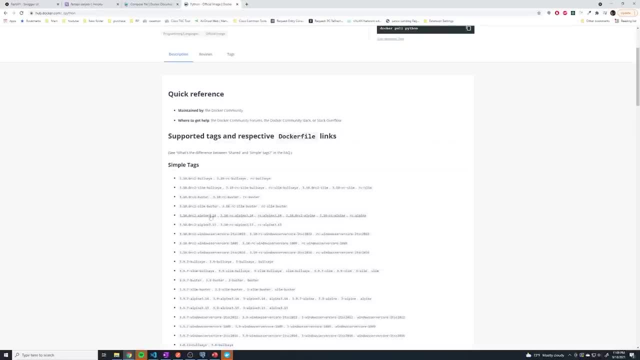 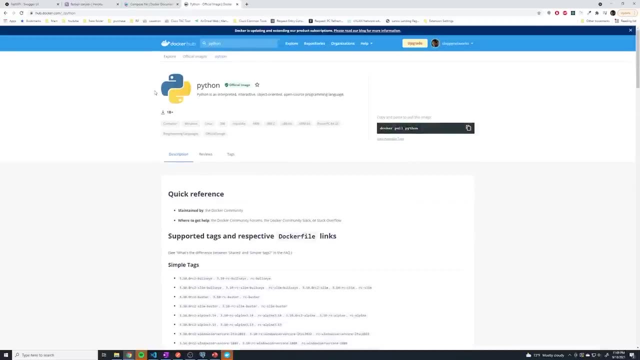 that we could pretty much ever want, And then they got slim images. they got the Alpine images as well, But we're going to use just the standard image. Now, if we use this specific image, the problem with this is that this is just a basic image with Python. there's nothing else on it, And at that point, if 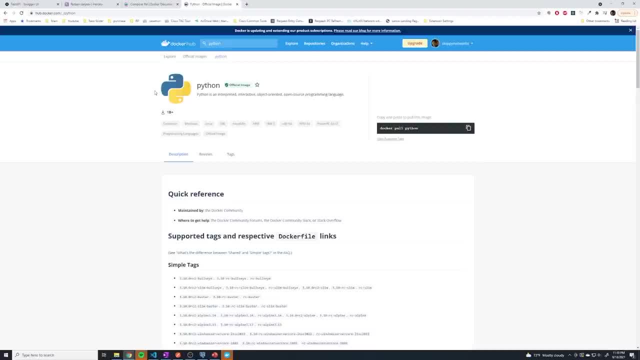 we just have a basic Python container, then we have to do all of the work of copying our source code onto the Docker container And then we have to install all of our dependencies and set up our application. And that kind of defeats the purpose of Docker, Because 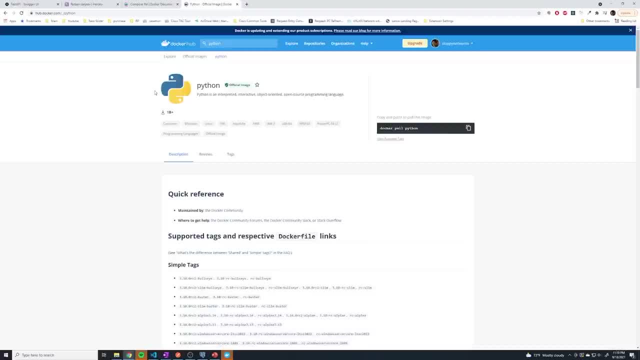 the main idea behind Docker is that we actually create an image that has everything that we need to run our application. So we just start up the image, Or I guess we technically start up the container which is made from the image, and that should just have everything it needs. 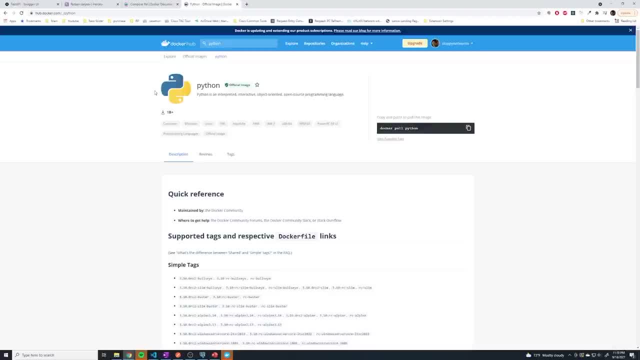 And it should just start working right away. So that's exactly what I want to do, And to actually get that accomplished, we're going to have to create our own custom image, And all custom images need to start off with a fix image. So we're going to start off with 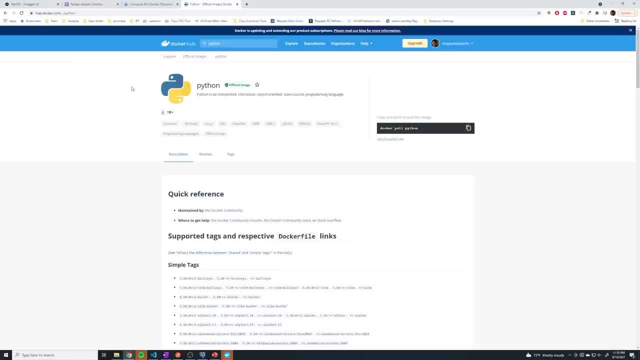 this base Python image And we're going to customize it by doing a few things, including copying our source code into it And installing all the dependencies. I've already run the fifth one. Now we've kind of come up with something which is just here. OK, now let's. 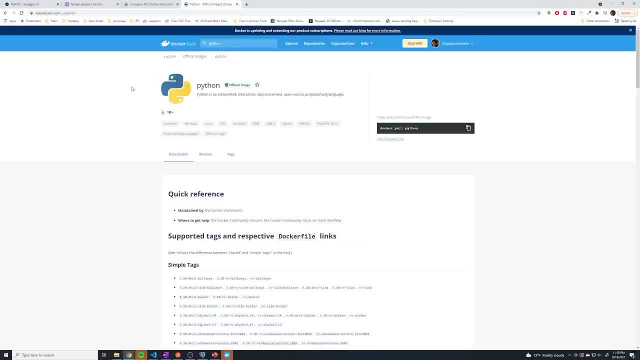 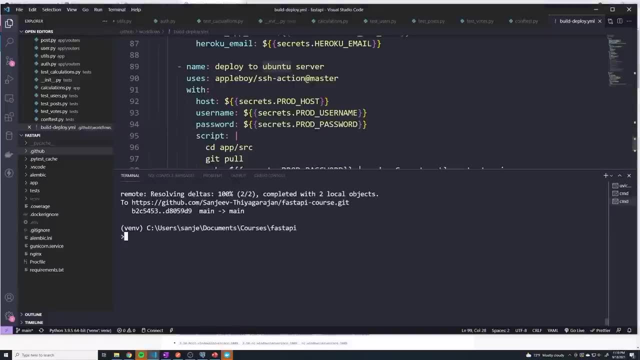 launch our robot. Let's get started. All right, so this goes over to imm Zhongla and let's just dependencies and setting up a few other details. So to actually create a custom Docker image, we're going to go to our project directory And we're going to create a file that's referred to. 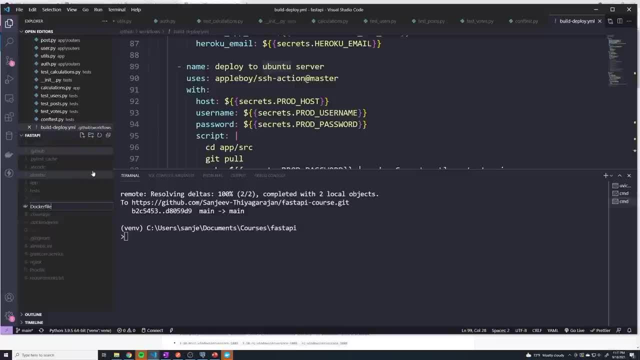 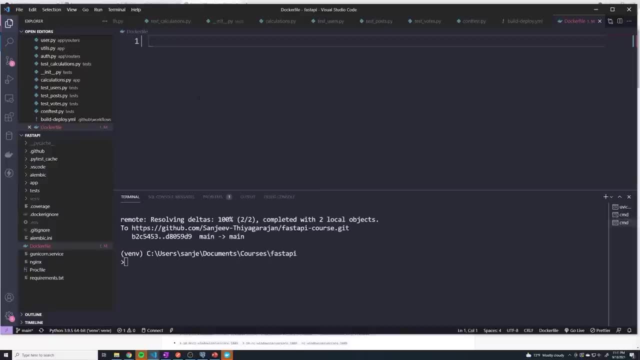 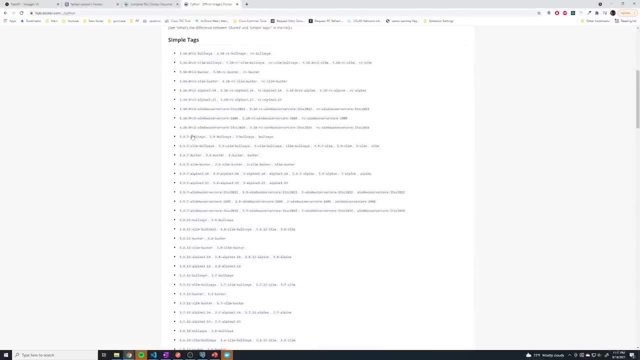 as a Docker file. Now this Docker file is going to have all of the steps necessary to create our own custom image, And the first thing that we have to do is we have to set up or specify our base image. So we're going to use this Python 3.9.7 image as the base image. So what we do is we say: 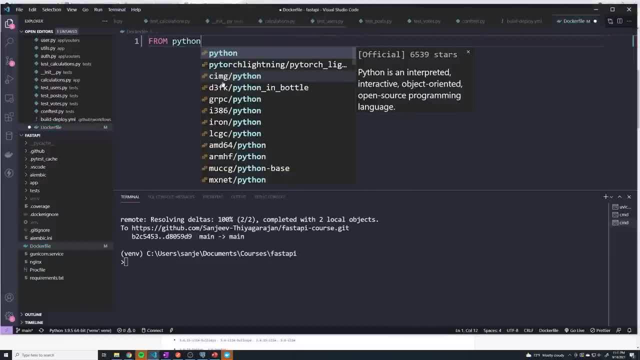 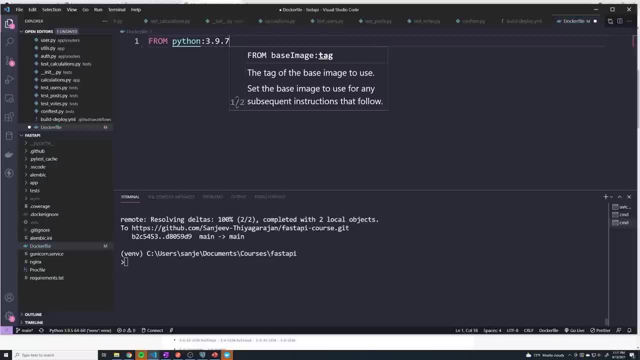 from and then the name of the image. So this is the Python image And then, if we want to, we can also do a version. So I'm going to do 3.9.7.. If you're wondering where I'm getting this from. 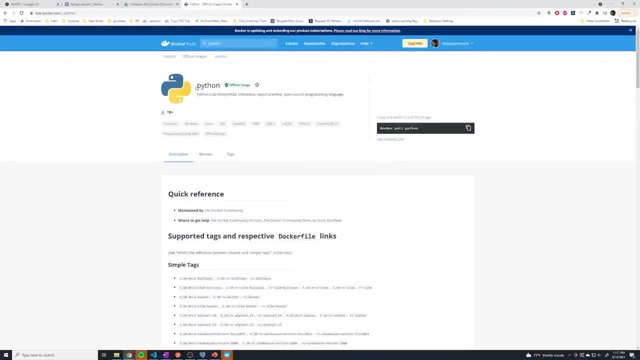 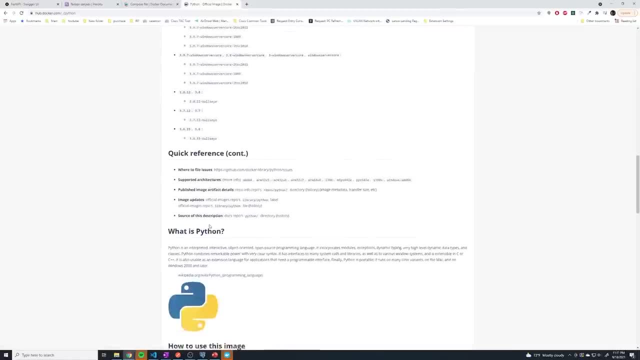 this is all from the documentation. you just say from the name of the image, which in this case is Python, And then you can see the different tags. So if you want 3.9.7 slim bullseye, that you got that, And if you want to see them, 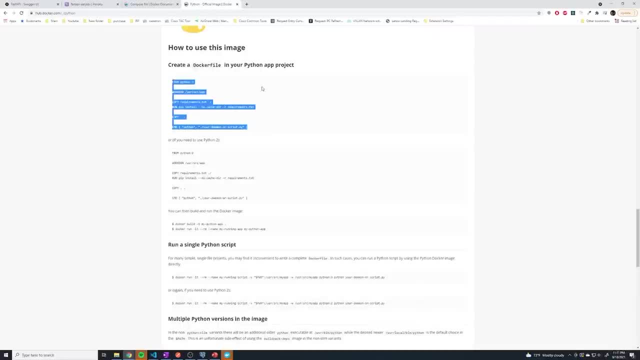 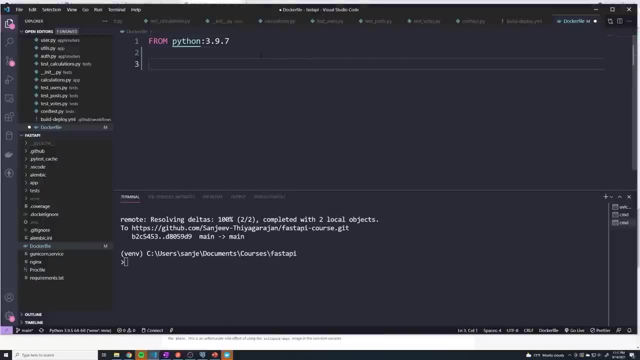 going over that in an example. we're kind of basically just following this. essentially, The next step is going to be an optional step, But I always like to do this. we're going to use the workder flag And this is going to set the working directory. So I'm going to say this is going to be. 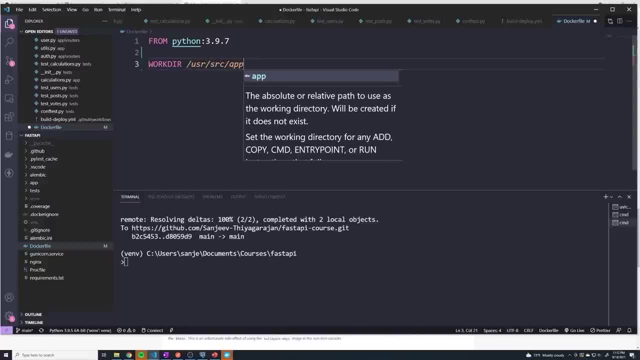 users source slash app. Now, how do I know that there's a folder called user slash source? I've actually run the Python image myself And I checked to see where I could actually set up my application. So I found that there is a path here, And then I want to create a folder called app, And this is where I'm going. 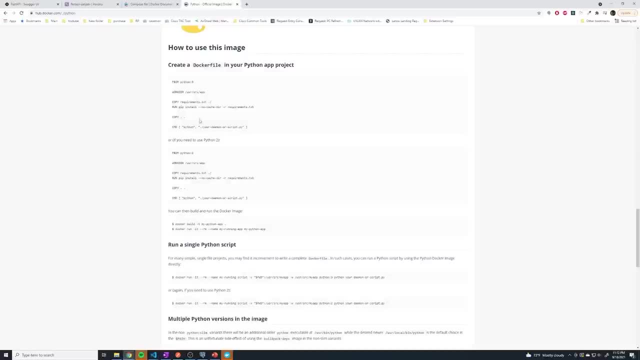 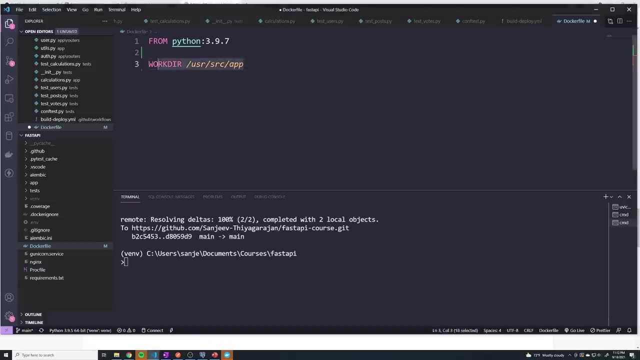 to store all of my application code And, once again, you can take a look at the documentation and it does the same thing. So if you ever lost, just take a look at the doc and it's going to help explain things. But, like I said, this is the optional command in this case, because what it 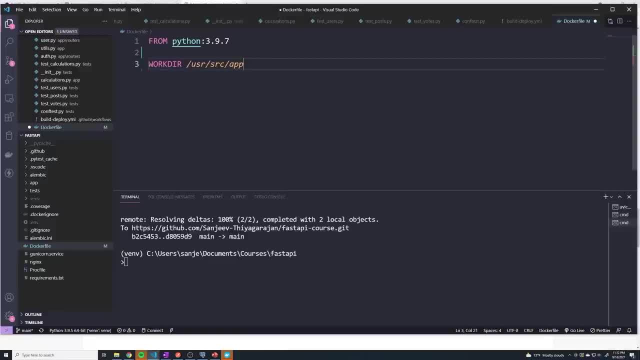 really does is it's going to tell Docker this is where all of the commands are going to essentially run from. So it's like doing a CD into slash user, slash source, slash app, And then, anytime we give directions, it's always going to do everything in that directory. So it's just going to help. 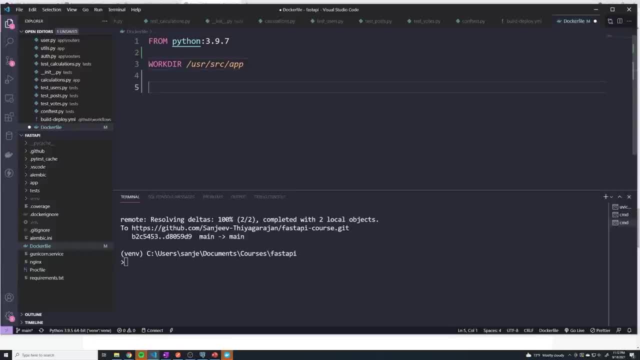 simplify some of the later steps, But it is technically optional. The next thing that I want to do is I want to copy our requirementstxt file from our local machine onto our Docker container. So we use the copy command. We see we want to copy requirementstxt, And then we have. 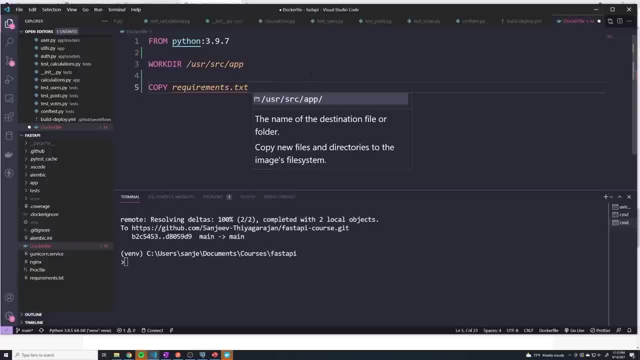 to specify the directory within our container or image that we want to copy it to. So I'm going to do that slash. So where does this exactly point to? Well, remember, we set our working directory, So everything is going to be with regards to that directory. So when I say the current directory, 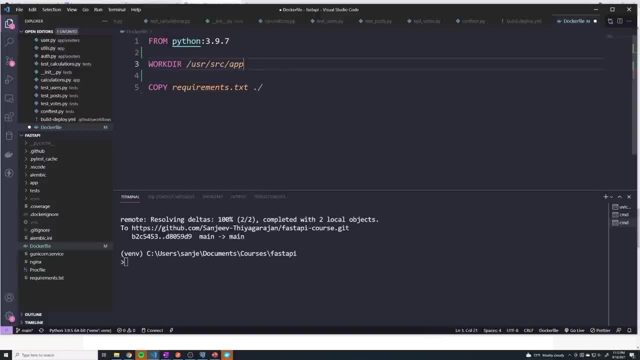 that means this directory. Now, if we didn't have this line right here, then we would have to specify the full path to that directory. So you can see that it's kind of simplifying things for us, Because then we can just kind of say, Hey, I want to use the current directory, because that's. 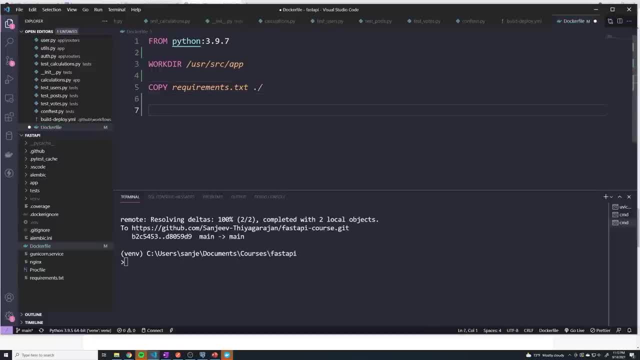 what the working directory is, And the next thing that I want to do is run a command which is going to be responsible for installing all of our dependencies, because we have our requirementstxt file copied into our Docker container. So we're going to do a pip, install The dash r and then 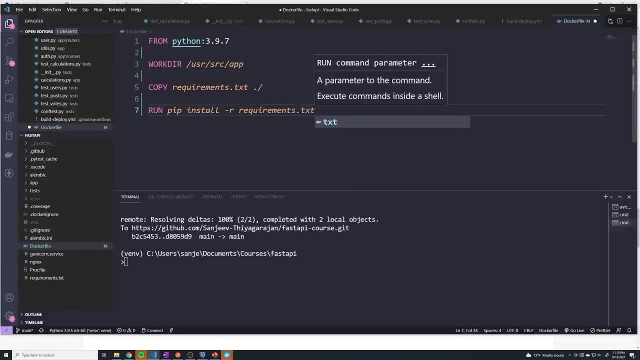 requirementstxt And, if you want to, we can also specify the dash dash, no, dash cash, dash der, if you wanted to as well. And so that's going to install all of our dependencies. Then the next thing that I'm going to do is I'm going to do copy Dot dot. So what does this mean? this is going. 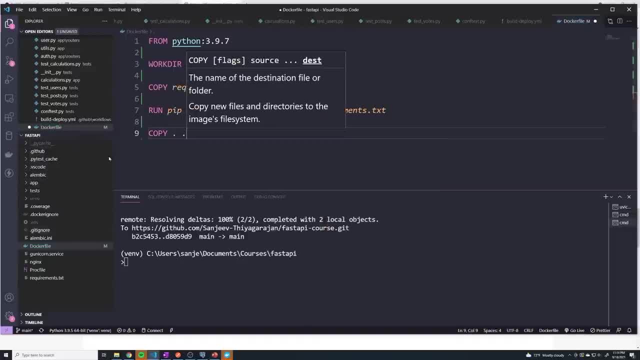 to copy everything in our current directory, So all of our source code, and then it's going to copy it into the current directory in our container. So what is the current directory? Well, that's the one that's set by work there And, once again, if we don't have this defined, then we would have to. 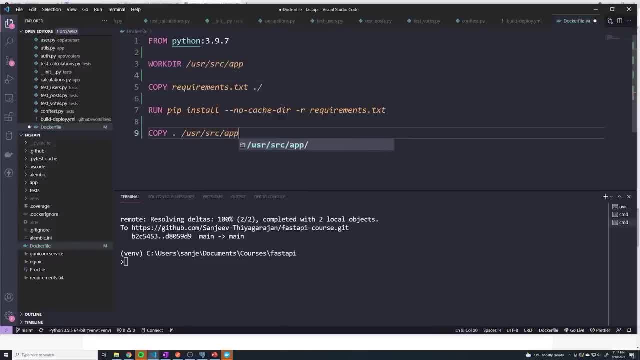 specify the full path of slash user: slash source- slash app. Now, one thing that you might notice: that we copy all of our source code at the end right here, which is going to include everything in our directory, including the requirementstxt file. So you might be wondering, well, why exactly? 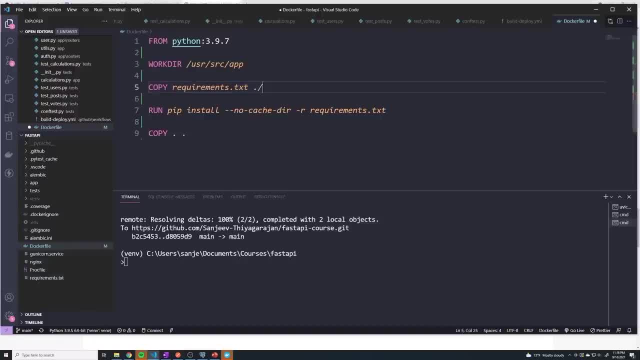 do we copy just the requirementstxt file up here? Well, this is a little bit of an optimization that doctor, that Docker provides us. So when Docker runs, when we build images from a Docker file, it actually treats each one of these lines or steps as a layer of the image, So kind of builds. 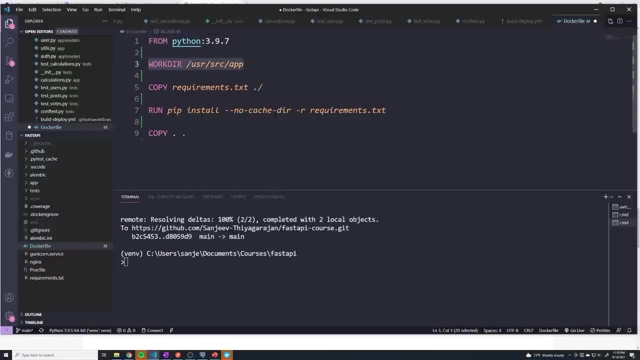 an image by running the first layer, Then creating the second layer, the third, fourth and fifth layer, And it actually caches the result of each step. So this is important because when you cache the result, if nothing changes, then we can just use the cache result. So let's say I, you know, run this image or I create an image from 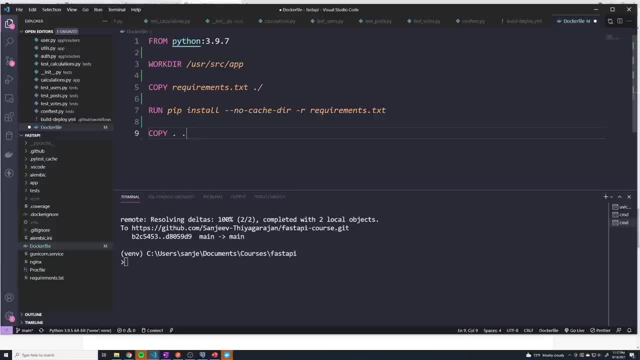 this file. It's going to take a certain amount of time because it has to. it has to do a pip install requirementstxt where it's installing all the dependencies, which does take a decent amount of time. But if I run this again, 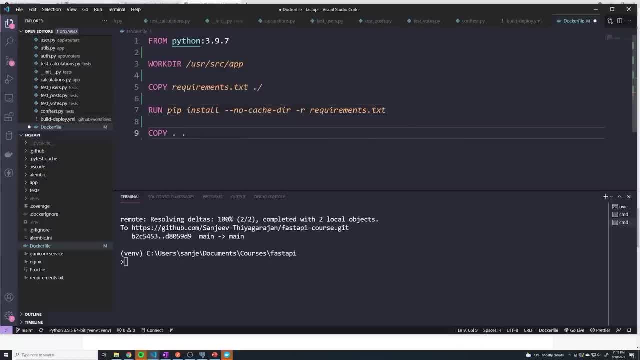 right and nothing changes. well then it can just use the cache result because it knows nothing's changed. And this is important because when I change my source code here, maybe like my databasepy file, it's going to see what steps changed right. And so if I change my source code, 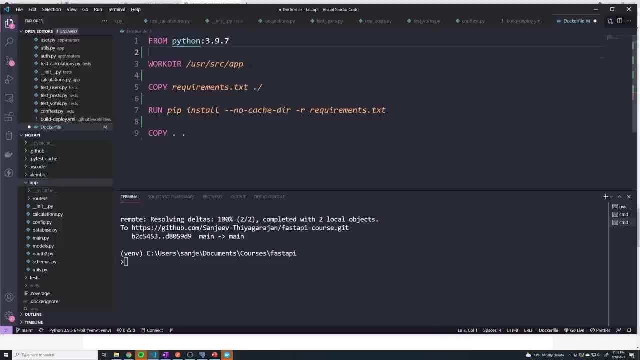 does that change the base image? No, we're still using the same base image. Does it change the working directory that we used? Nope, still the same. Did it change the requirementstxt file? Nope, still the same. it change any of the dependencies that we installed? Absolutely not. It only changed. 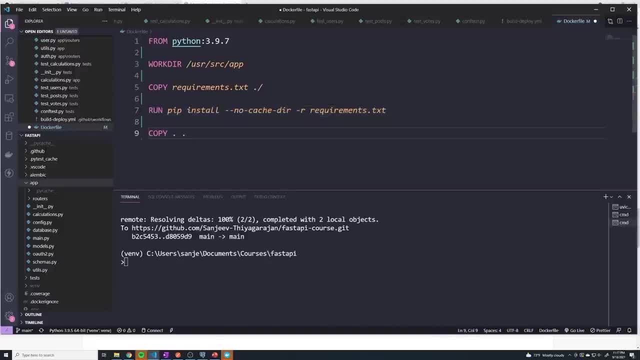 the final step. So this causes Docker to be able to use the cast result of step one, two, three, four of step four and it only has to rerun step five. But if we change requirementstxt- this file right here, then it knows that this step changed here, So it's going to have to. 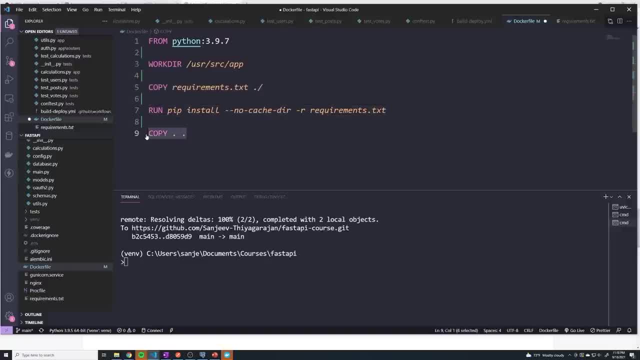 rerun this step, then this step, then this step. Right, And so this gives us an advantage, because anytime we change our source code, we only have to run this last step, And if we change our requirementstxt, then we have to run all of these steps And keep in mind that this step is. 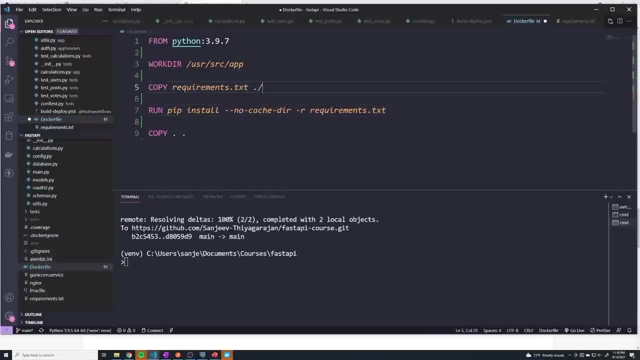 the longest step. And so if I had actually like- if I can comment this out- so if I didn't have this line and instead I copied all of my source code right here, what would happen is, every time I changed any code, I would have to rerun this step. And so this gives us an advantage, because 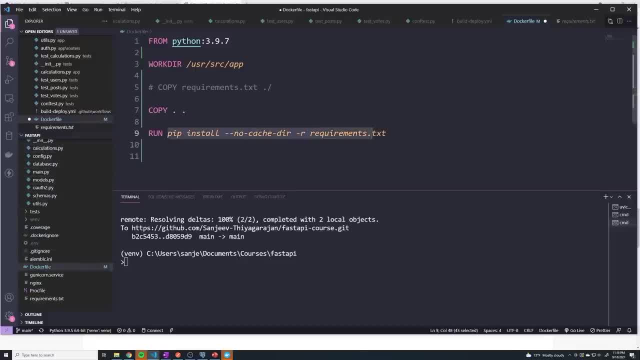 in any of my files. I would have to rerun a pip install every single time, And that would cause us to have to rerun the longest step in our build process, And so that's why we have this optimization, That's why we copy the requirementstxt file, so that we can cache that result. 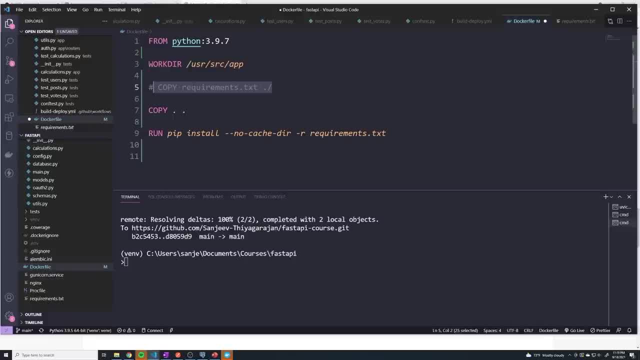 And so anytime we make any changes to that file- sorry, anytime we make any changes to our source code that's not in that file, we don't have to rerun a pip install, All right. And then, finally, we have to give it the command that we want to run when we start the 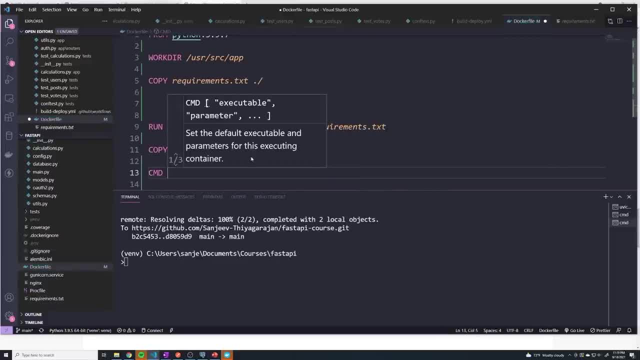 container. So we'll say cmd brackets, And so the command that we want to run is uvcorn, appmain app. And so the way we actually specify the command is we break out each word of the command. So here we do uvcorn, And then we say appmain app. And then here we're going to. 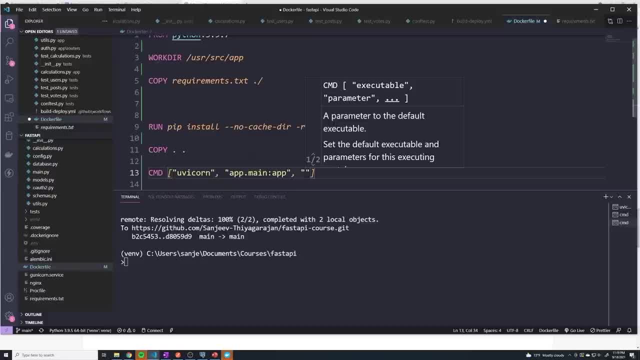 pass in the the host flag and the port flag, like we did on our Ubuntu machine. So we do dash dash, host 000.. And we do dash dash port, That's gonna be 8000.. Okay, so it's basically anytime you have. 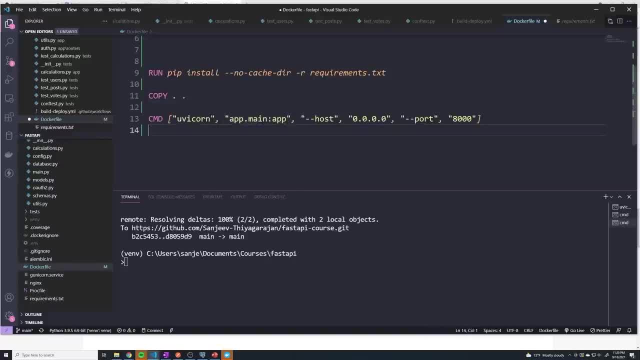 a space between the commands, you just split it up into a different string within this list. That's just kind of the syntax that you have to use with these Docker files, But it's the same thing as running uvcorn appmain app and then dash, dash, host. 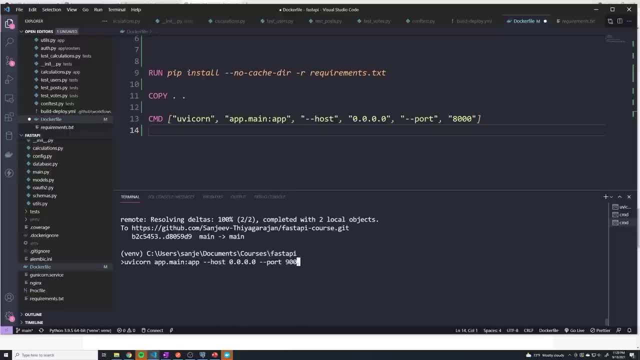 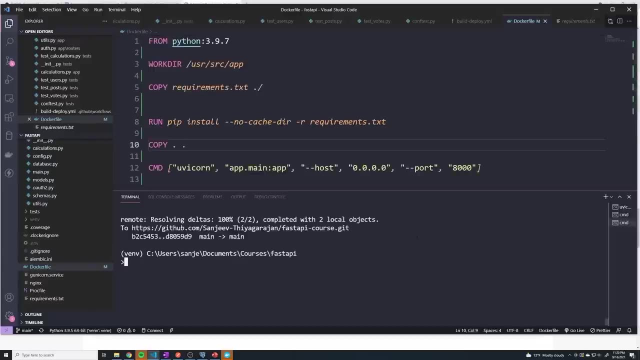 dash, dash, port, 8000, 8000.. So it's just going to essentially run this in our container. we just have to provide it in this format, All right, And so now our Docker file is complete and we can actually build our image. So what we're going to do is: I'm going to do a Docker. 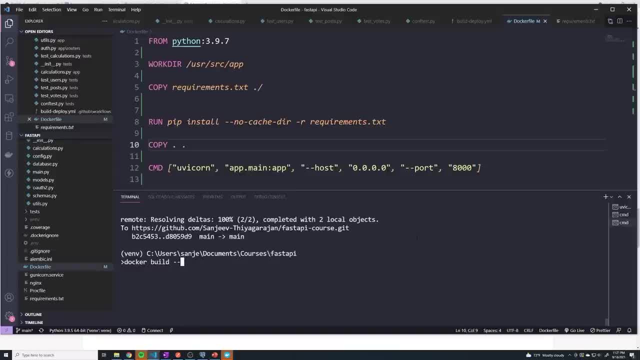 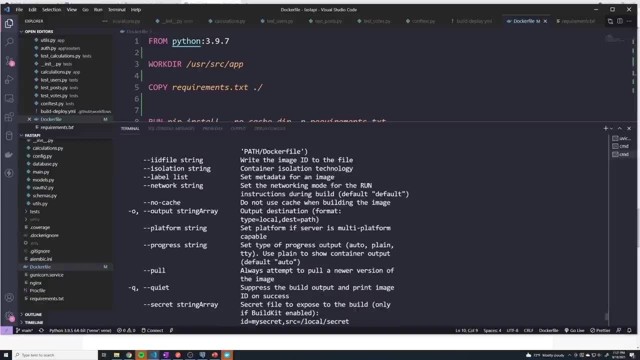 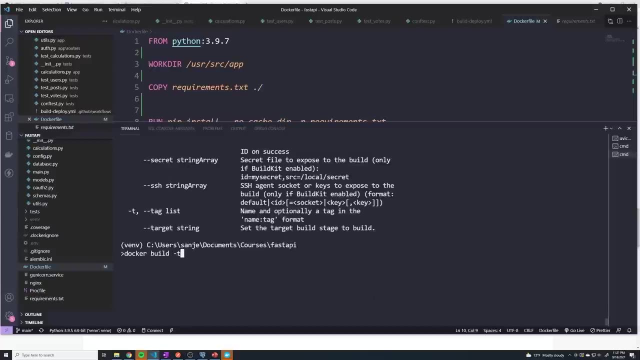 and then the command to build our images, build. And then we'll do a dash, dash, help. So we can see all of the different flags. And most of these don't really matter. The only one I really care about is a tag, So I want to give this a name. So I'm going to say Docker, build, dash T. I'm going 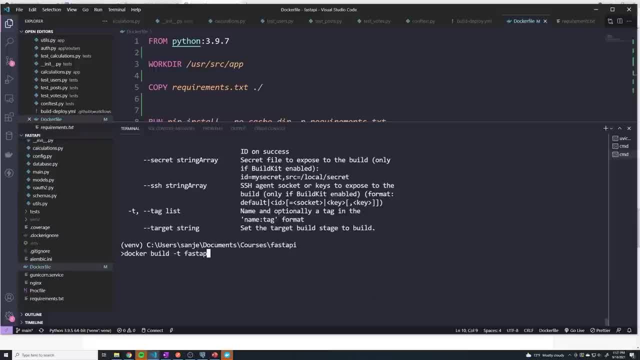 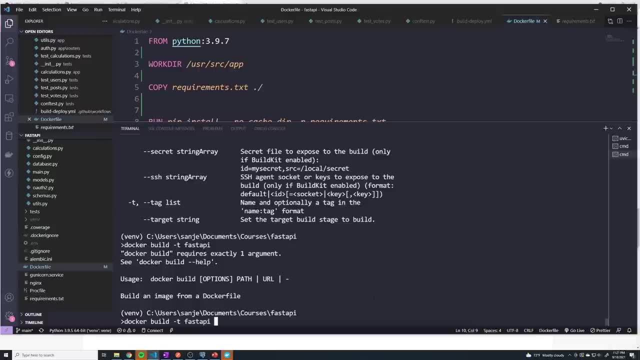 to give this image- water- a name that I think is reasonable. I'm just going to call this fast API, And we have to pass in one last argument, which I forgot, which is going to be the, the context you can think of. the context is just kind of the directory. 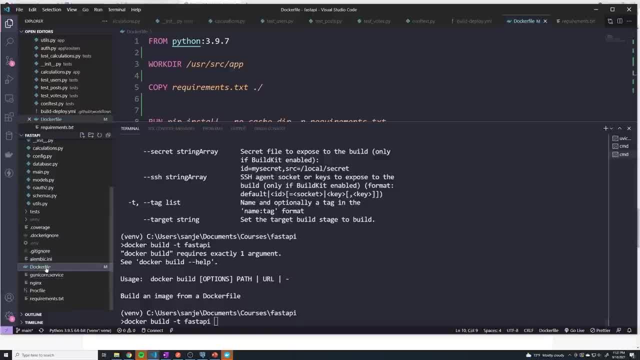 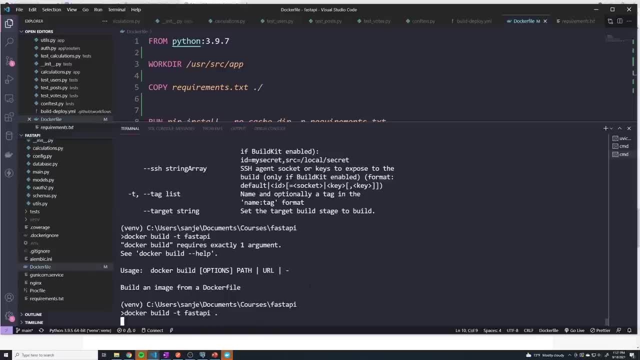 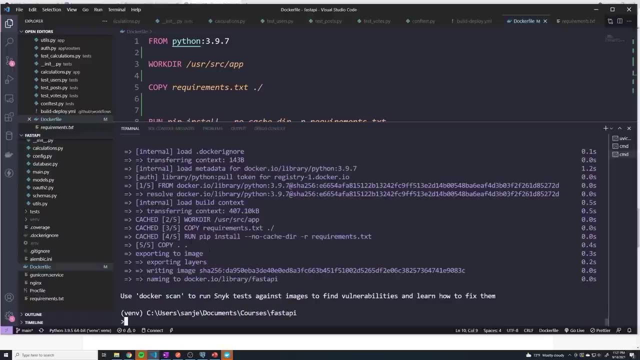 where the Docker file is. So it's going to be in the current directory because we can see the Docker file is in the root of our folder structure. So I can just say dot. And so now it's actually going to build our, our image, And if I do a Docker image, LS, 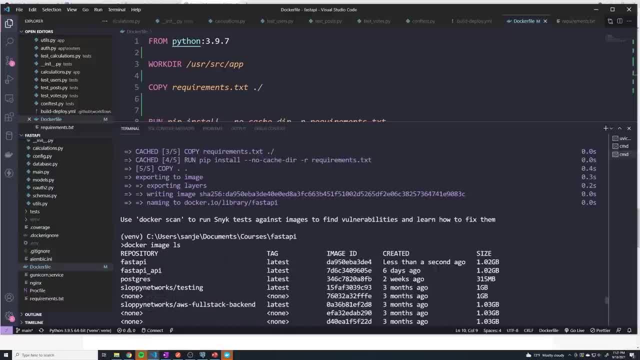 we can see all of our Docker images and you'll see that I've got a whole bunch, But we've got my fast API right up here And so now we can go ahead and use it outright in Docker- this image for actually building out a container- And we can run a whole bunch of Docker commands. 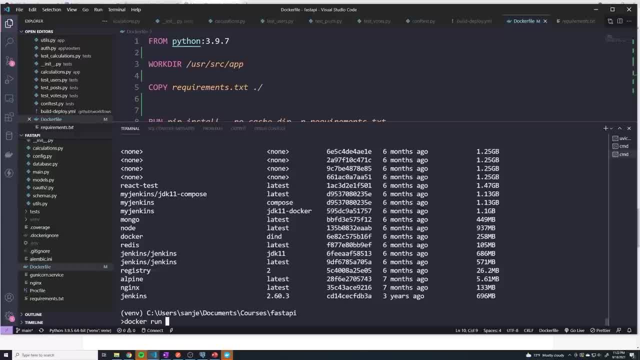 like Docker run and then specify the image- image that you want to use- and then pass in all the flags. But I don't like doing that. I don't like working with Docker run. Instead, I want to use Docker compose, And if you have never worked with Docker compose, Docker compose. it does the same. 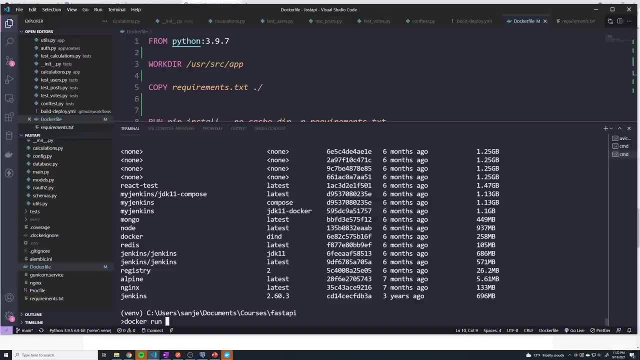 thing as running Docker commands on the CLI. we just provide all the instructions on a file so that we don't have to remember all of these long commands With all of these extra flags. we literally write out the flags in a file And then we can just say Docker, compose up, and it's going. 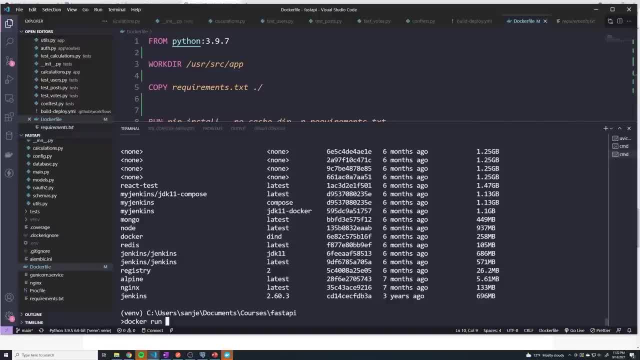 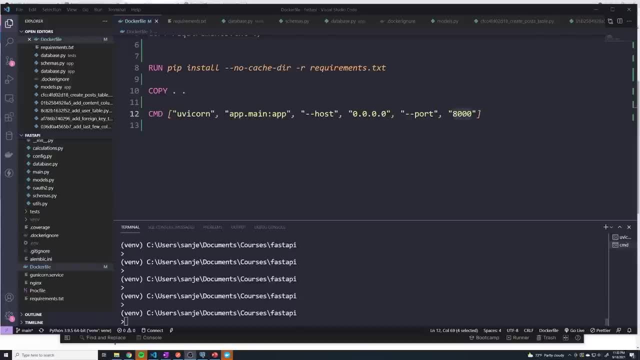 to bring up all of our containers. So we're going to take a look at Docker compose in the next video and see how we can get that set up. Alright, so we're going to learn about how we can use Docker compose to automatically spin up our containers with the desired configuration, And it's good. 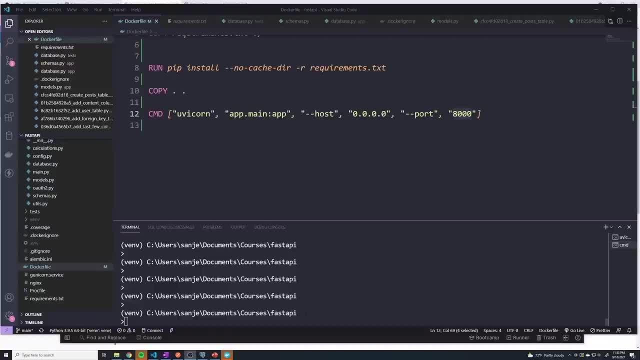 you're going to see that it's so much easier to use Docker compose than just running Docker run whenever you need to, because we can spin up multiple containers all with one command And we can do that. So to use Docker compose, we have to provide the set of instructions using a file called. 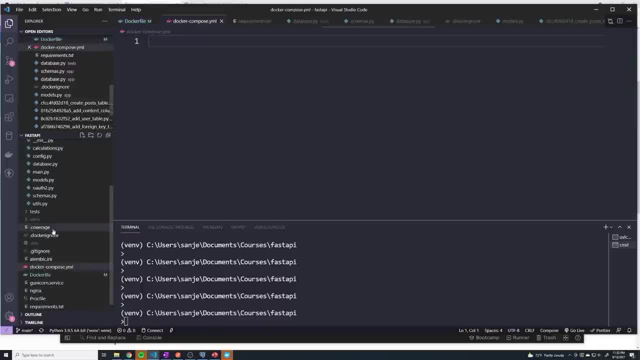 Docker dash compose dot YML, And so this is a YAML file, And if you don't know too much about YAML, it's just a, I guess technically like a markup language, I guess. But the most important thing to understand is that spacing matters. So this is kind of like Python, where you need to. 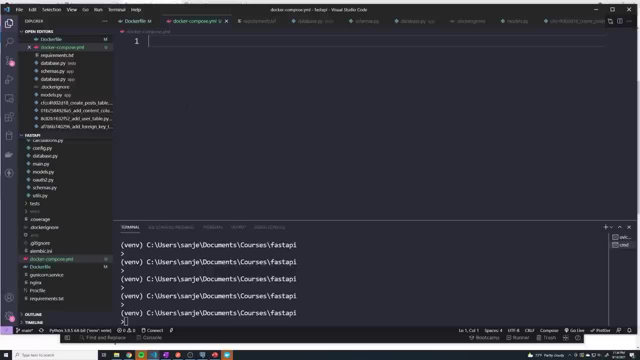 make sure that the tabs and the spaces are just right and everything lines up, or then it's going to start to throw errors And the first thing that we need to do is specify what version of Docker compose is. So we're going to need to specify what version of Docker compose is, And we're going to 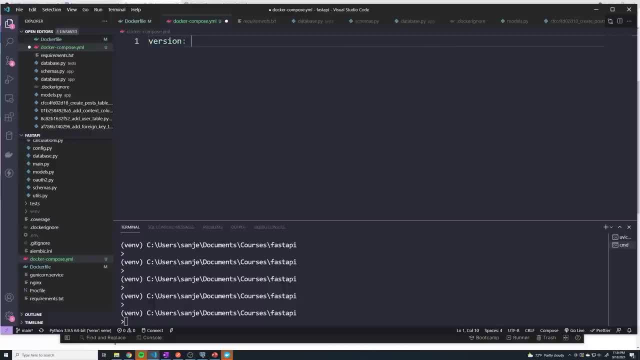 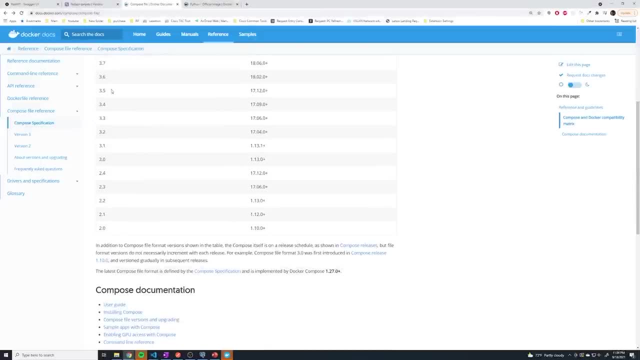 say version, And I'm going to say just version three. it's not the latest, it's just kind of most common one. If you actually go to the Docker documentation for compose file, you'll see the different versions that you can specify And you can actually take a look at the documentation and 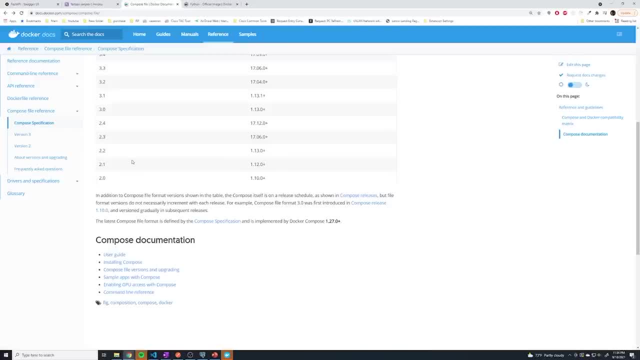 see what feature was introduced in what version, So you can figure out what version you need to perform all of your operations. We're not doing anything special, So version three is just fine for us. Then within Docker compose, we have a concept of services. 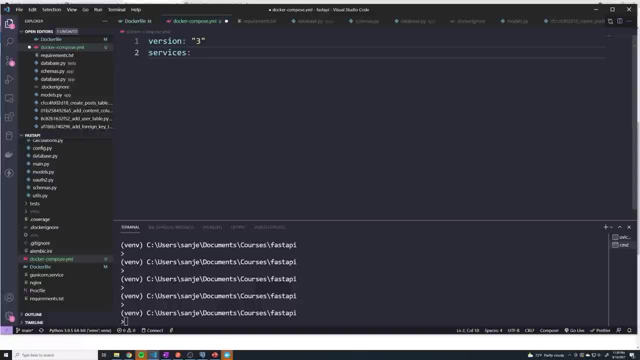 And so a service, really at the heart of it, is nothing more than just a container. So if you want Docker compose to spin you up a container, you have to define a service. If you want Docker compose to spin up four containers, we're going to have four different services, pretty simple. So we have to 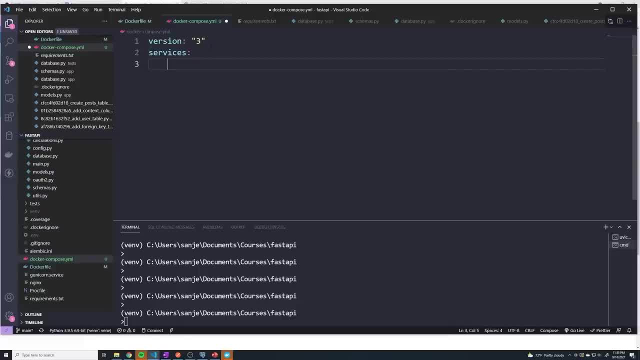 give each service or each container a name. So we're going to have one container for our fast API And I'm just going to call this container API or the service API, And the first thing that we need to do is we have to specify each container. So we're going to have one container for our fast API. 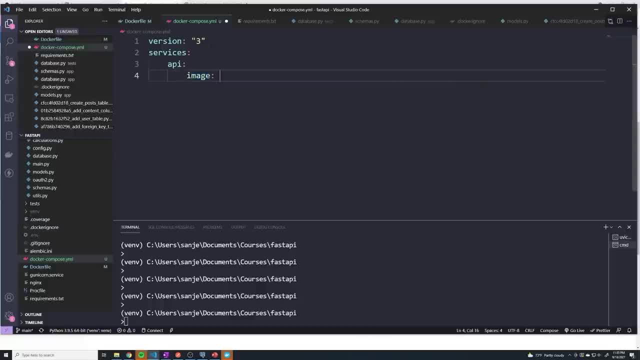 And then we can specify either the image that we use- So I could technically say like image, and then we can point to like the Python image- or I can specify build, where we can essentially do the same thing that we did before in the previous video, where we ran a Docker build and then 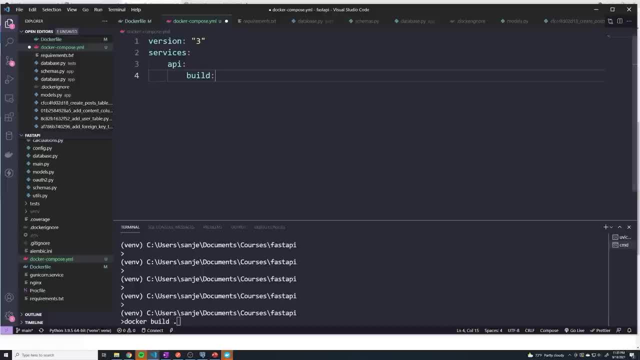 provided the location of the Docker file. But we can just specify that here within Docker compose, that Docker compose will automatically build the image for us if it doesn't exist. So we'll say Docker build and then we specify the context of the path to the Docker file. 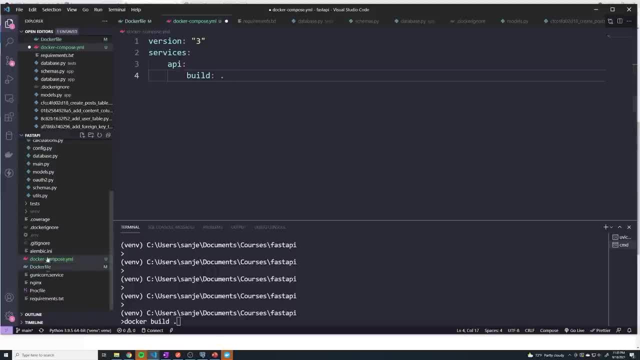 which is the current directory based off of where the Docker composes. So they're in the same directory. So I just say current directory, And then we have to specify a port that we want to open up, because this is an API, So the outside world needs to be able to reach our container. But 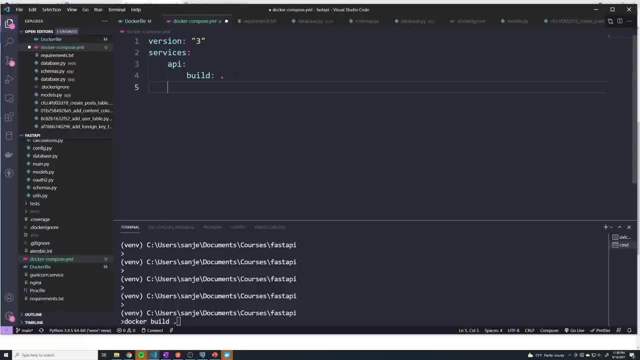 by default all containers can't talk to the or sorry, by default that the outside world can't actually talk to your container. So we have to open up or poke holes on our local machine to open up some ports. So we say ports and this expects an a. 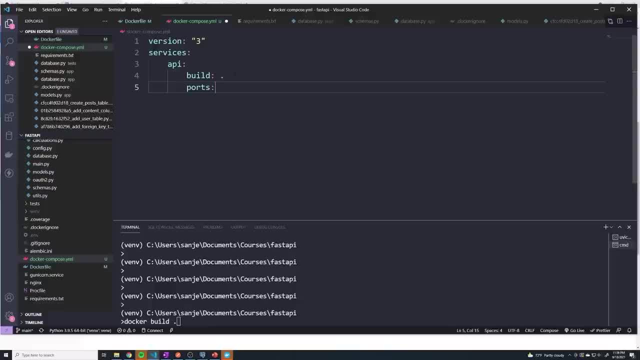 an array of ports, And so there's two different ways to do: an array With YAML or with a Docker compose file. we can do, you know, just an array like this, where we just provide a list of things. Or we can also do it like this, where we do a dash and then provide you know something and then a. 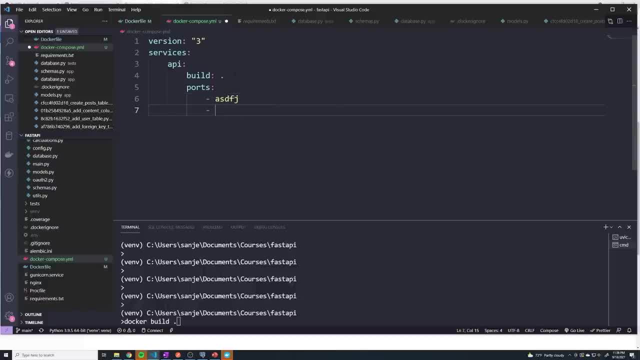 dash for the next entry in the list. So I'm going to use this syntax because I kind of like it better. But to open a port, there's a specific format that we're going to use. So what we say is: there's gonna be two numbers, there's going to be the. 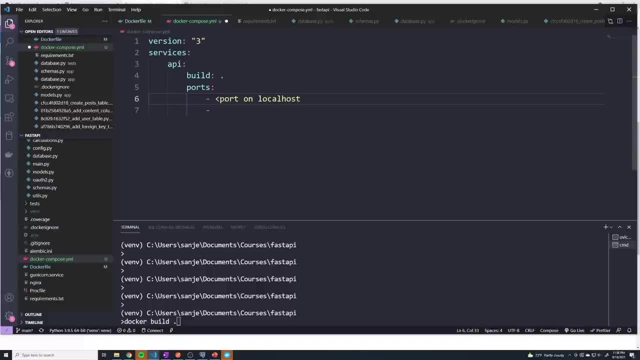 port on local host, And then we do that, And then we do the port on container. Alright. so what's essentially happening is we're telling Docker, if we receive traffic on our local host on this sport, this port specified here, we're going to forward it to this specific port on the. 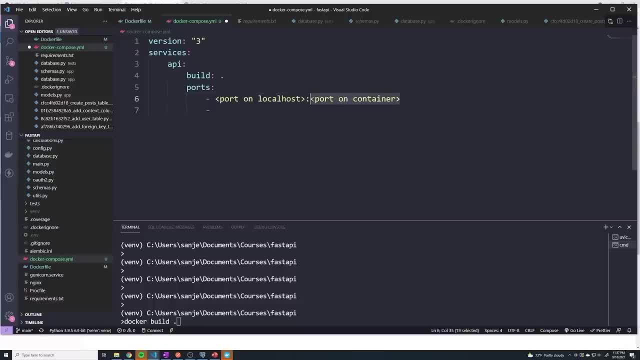 container. So the second number is a little bit easier to set up because it's going to be whatever port our applications running on. So if we take a look at our Docker file we can see that our container is going to be listening on port 8000.. So we want to set this second number to be port. 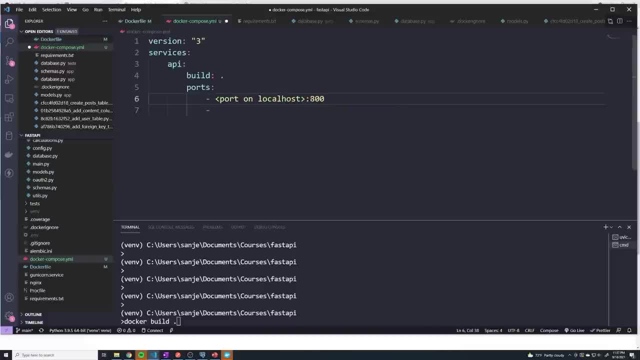 8000.. And keep in mind you could choose to use any other value. So if you decided to use port 80 here, then you would just change it to port 80 here, But I'm gonna leave it as 8000, just for. 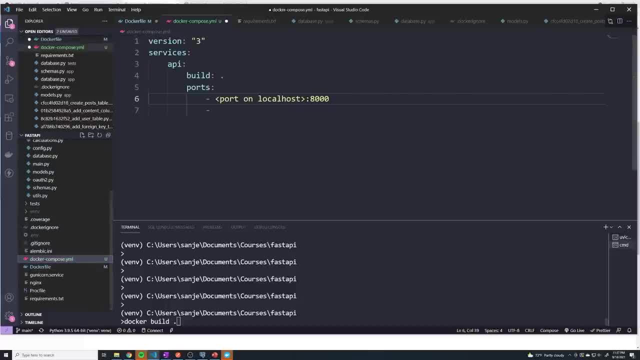 simplicity sake, Then the second number that we're going to use is going to be the port on the local machine or on the local host, which in this case is my Windows machine. But if it's on the production server it's going to be whatever machine or IP of that specific servers, And so 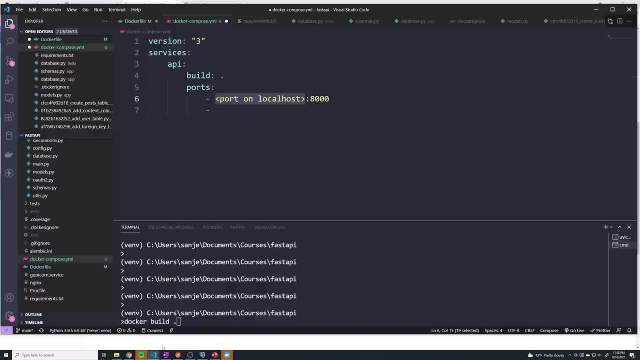 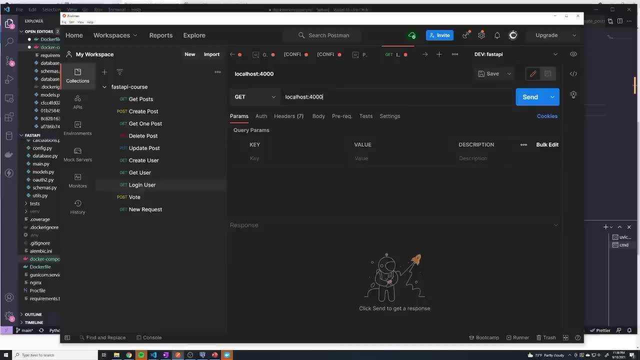 here we could specify any ports if you can literally pick any port that's open. So if I said port 4000, what that means is that you know, if I go to my, my postman, this would be the equivalent. 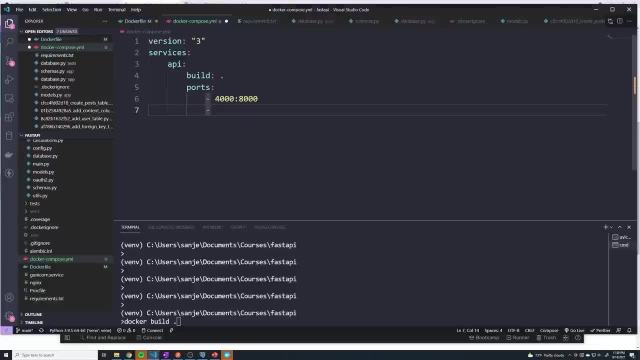 of doing localhost colon 4000. Right, which is that first number. And so anytime we send traffic to that specific port on a local machine, it's going to route it to port 8000 in our container, which is what port our. 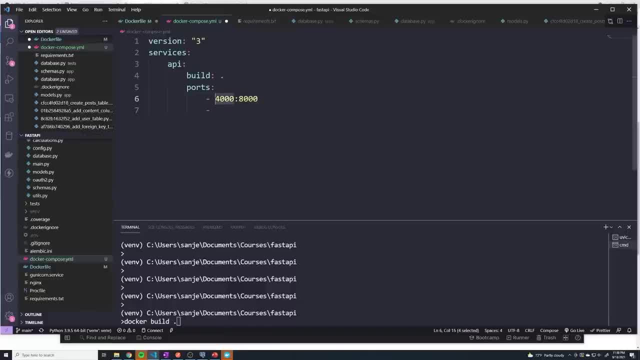 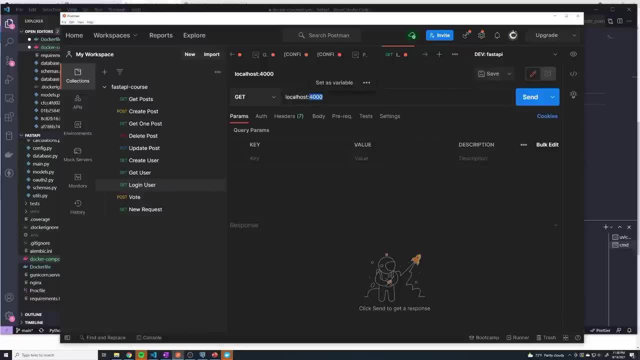 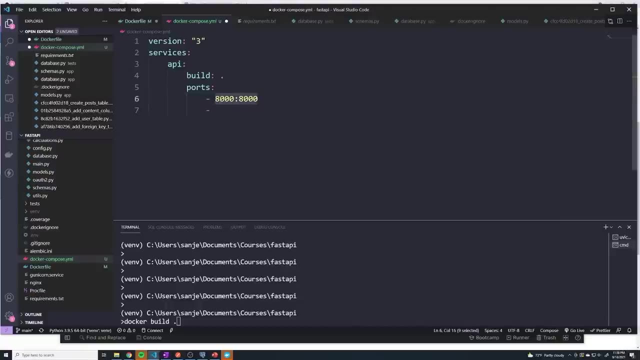 applications listening on. But if I change this to port 8000, as well, then our request would be localhost port 8000.. So I always like to have the two numbers match up, because it's just simpler. But sometimes that's not an option, So just pick a open port on your localhost machine. 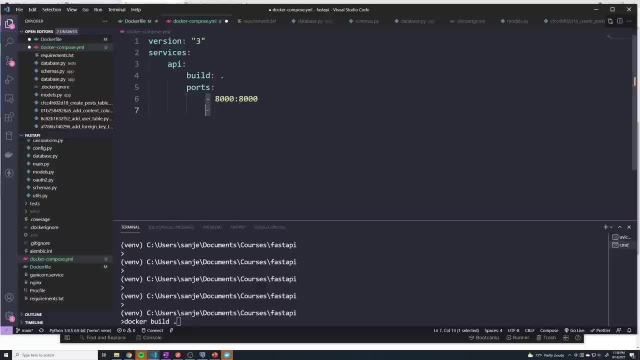 it doesn't really matter what it is, just make sure that you remember what it is. And I'm gonna leave it like that And I'll delete this line right here And for now, I think this is good enough, And what we're gonna do is we're going to try to run this and see what happens. So I'll say Docker dash. 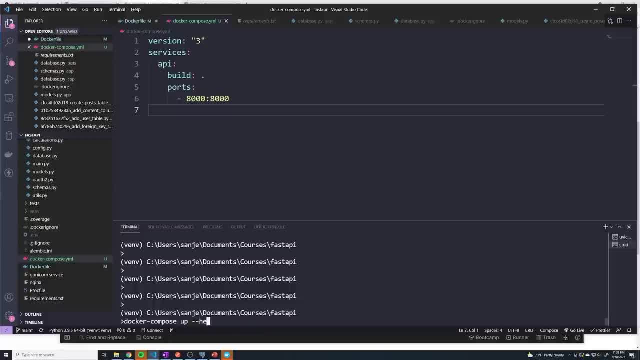 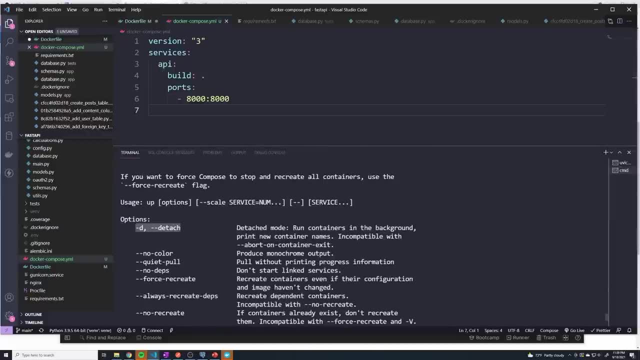 compose up And then, if I do dash dash help, we can see some other flags that we may need, And the only flag that I really need right now is the dash D. So this is gonna run the containers and in the background, so that we're not automatically connected to it. So I'll do dash dash. 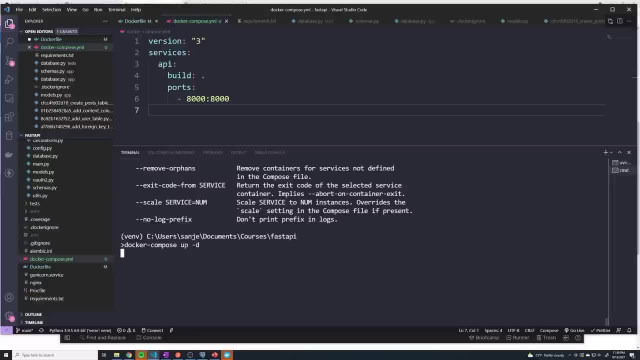 sorry, just dash D Right. And so you'll see, if you take a look, what's happening is we're rebuilding our image. So you'll see, if you take a look, we're doing this, We're rebuilding our image. 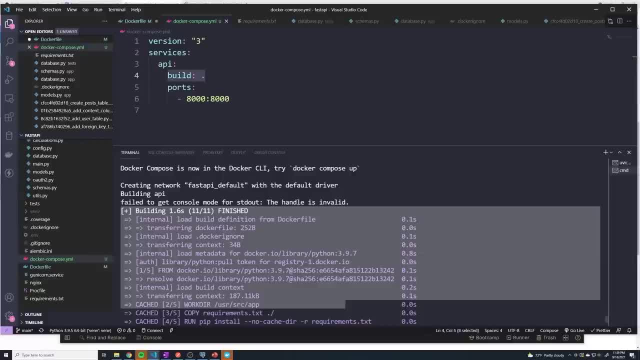 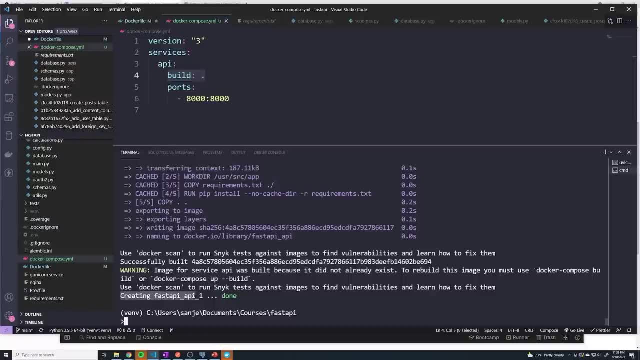 we're rebuilding our image. We're doing this. We're building this. We're doing this image. So, because we specified the build right here, it's going to build our image And then it's going to start our containers. So you can see that it's creating fast API underscore. 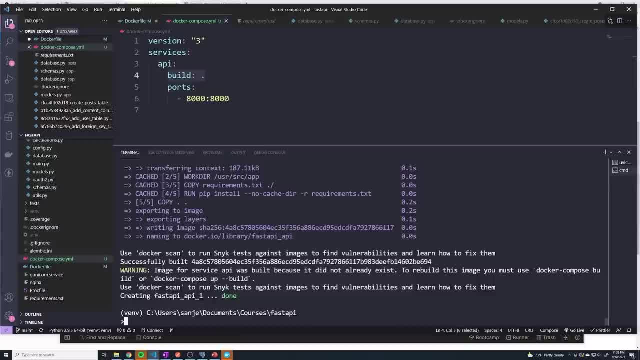 API underscore one, And so the the naming syntax comes from the project directory, So it's called fast API, Right? So that's why the first word. then we do underscore and the name of the service, So I call this service API, then it's API And then it has the number. 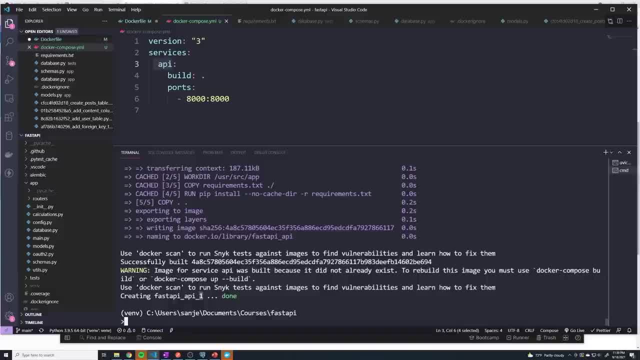 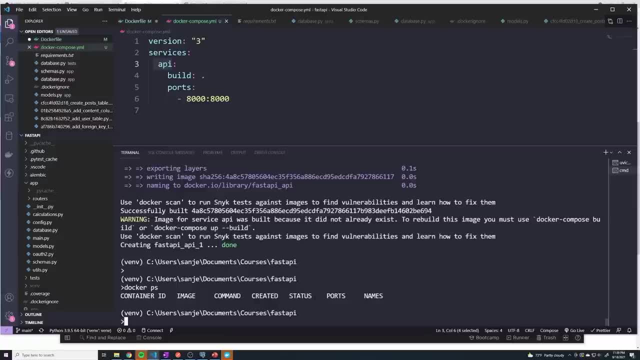 one because there's one instance. but if I told it to spin up four, then I'd have 123 and four. So we've got our container. If I do a Docker PS, we should be able to see. Nope, Oh, we can see it's down. And that's because if I do a Docker PS, dash a And we. 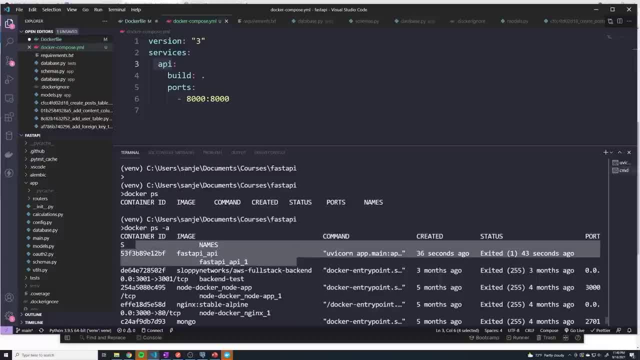 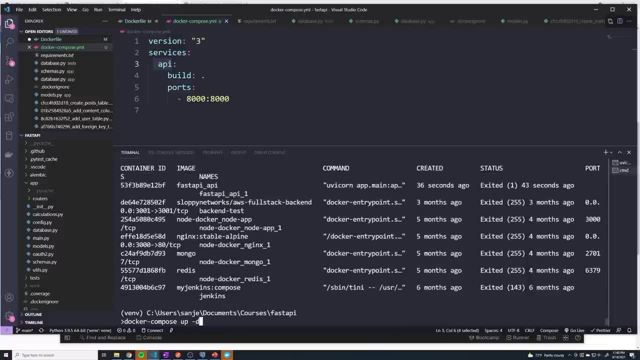 can see that this one right here Looks like it stopped 43 seconds ago And so it crashed for whatever reason, And that's okay. What we can do is, I think we can actually see the logs after it goes down. So if I do, Docker logs fast. 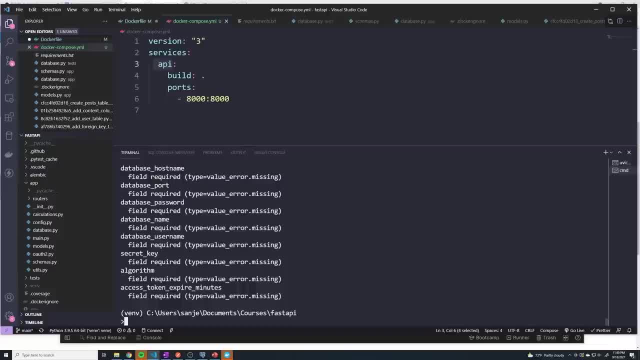 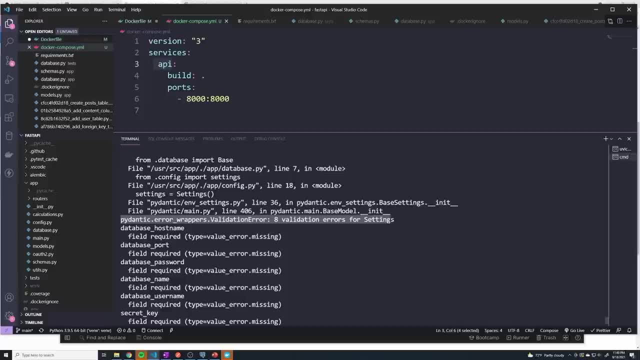 API one. we can actually take a look at the logs, at what caused it to go down, And we can see a couple things. But we can see that we get the pydentic error for our settings object, which is all of our environment variables. So obviously a container is like its own. 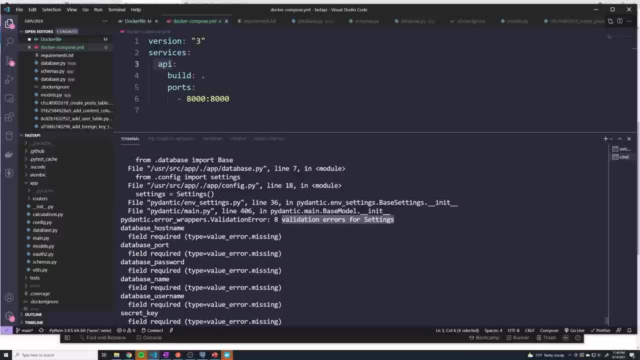 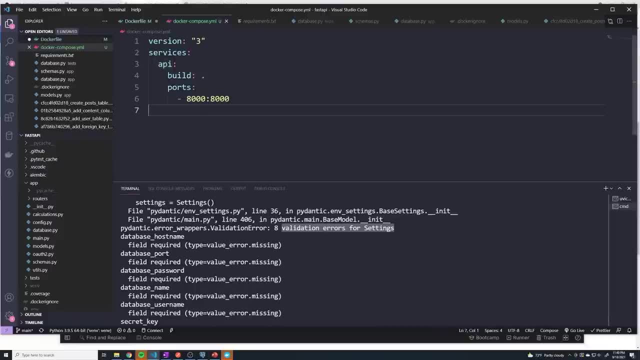 separate machine, So it needs all of the environment variables passed to it, or then our application is going to crash. So how do we pass an environment variable? Well, first of all we're going to need to have an environment variable in Docker. pretty simple, We just pass a environment field. 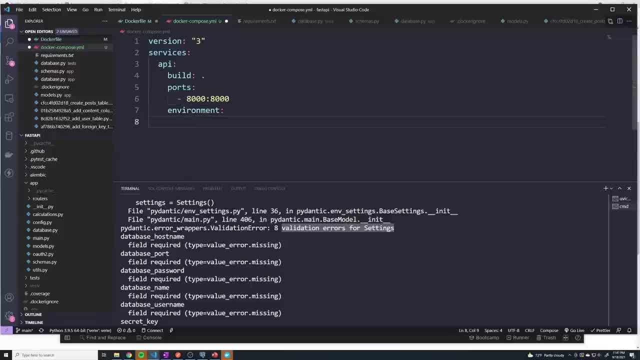 And then here it's going to provide a. you need to provide an array of environment variable, So I do dash, And then here we just specify our environment variable. So I'm actually going to copy and paste this section right here, And so these are all of our environment. 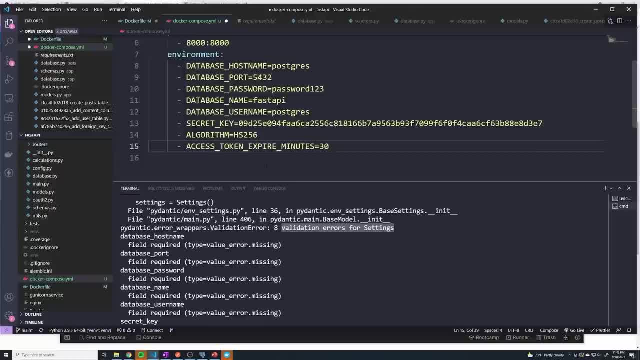 variables. Keep in mind, if you don't want to actually write out all of your environment variables, we can actually use Docker to point to aenv file or a environment file on your local machine. And if you want to do that, it's. 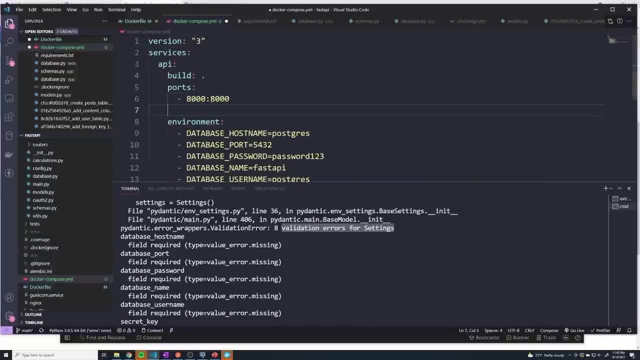 pretty simple Here. we would just specify the env underscore file And then you can actually provide multiple files. But in this case you just provide the path to the file. So it's going to be in the current directory And it's going to beenv. So you can do either. 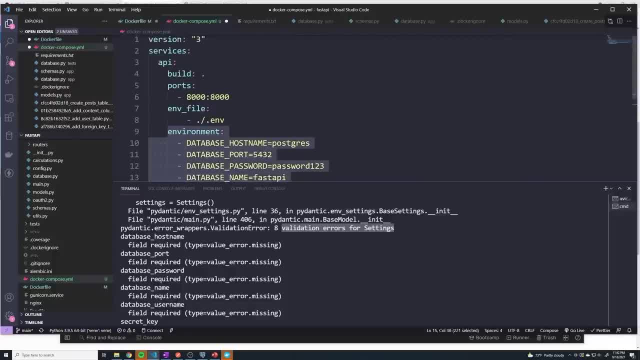 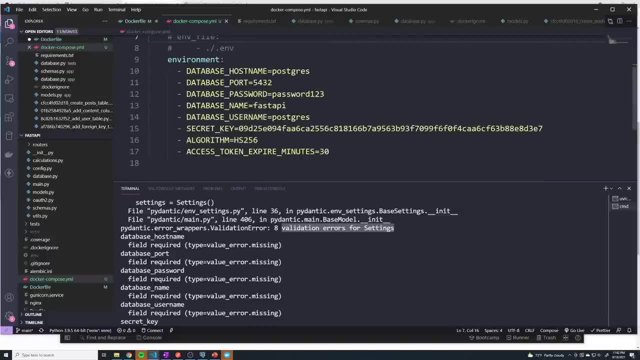 one or a combination of both. I'm just going to use this format so that we can see all of the environment variables, And I'm going to just comment this out for now, just for documentation purposes. And now what we're going to do is we're going to do a Docker. 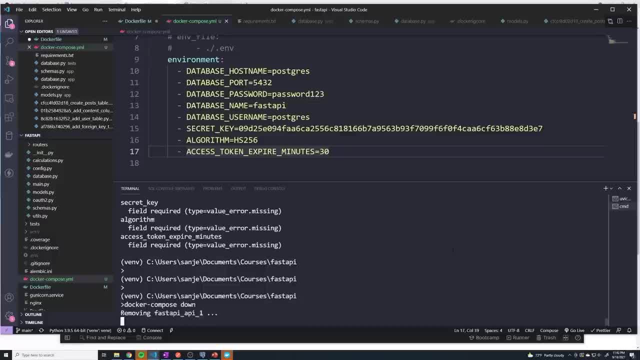 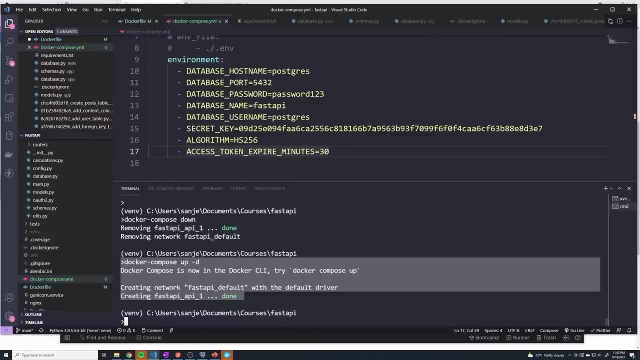 compose down, just to tear everything down, And I'm going to bring it back up and detached And notice, this time it didn't build the image. So why exactly didn't it build the image? Well, Docker Compose is very simple. All it does is it goes to Docker image, basically. 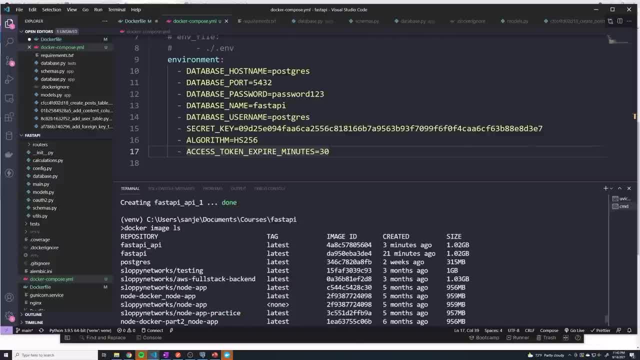 just runs a Docker image LS, And it looks for the image that it would have created And there's a very specific format that he uses, which is going to be the name of the folder or the directory and then underscore and then the service. So, since the image was, 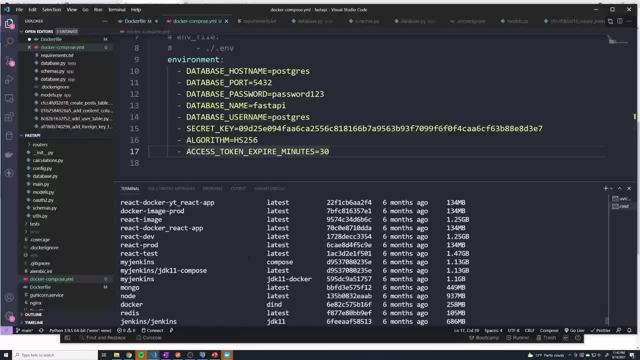 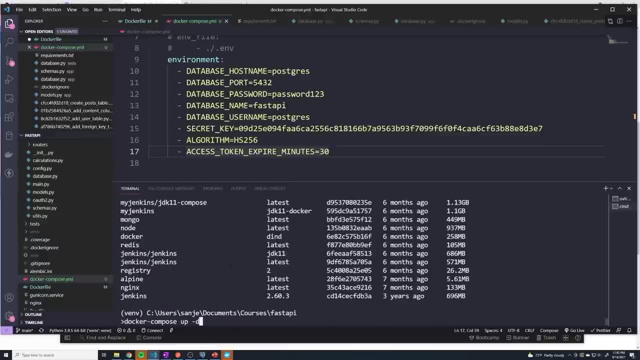 already created previously. it doesn't recreate it. However, if you obviously make changes to your, to your Docker file, and you want to make changes, then you would have to do Docker up And if you look for the flags, there should be a dash, dash. 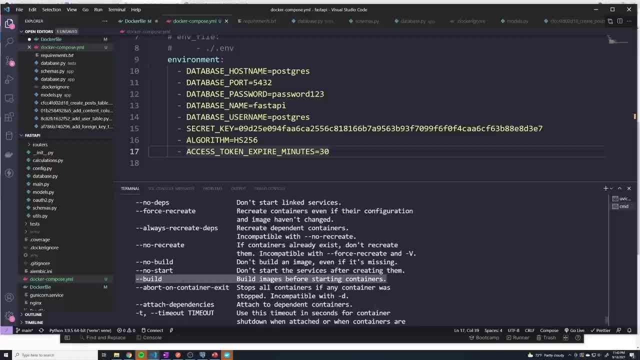 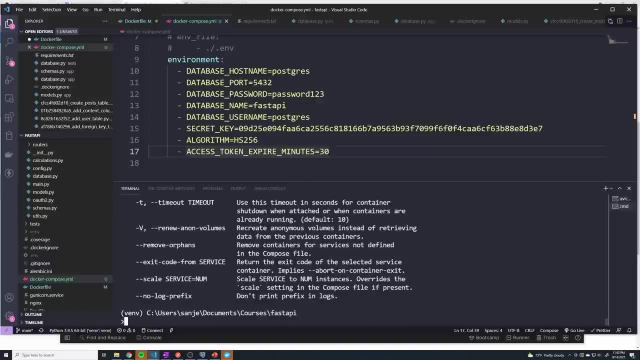 Let's see build. this is going to force it to build a new image. So keep in mind, anytime the the image has to change- and you've already, but the image already exists- then you have to pass in that flag to force Docker compose to let it know that, hey, I made some changes. 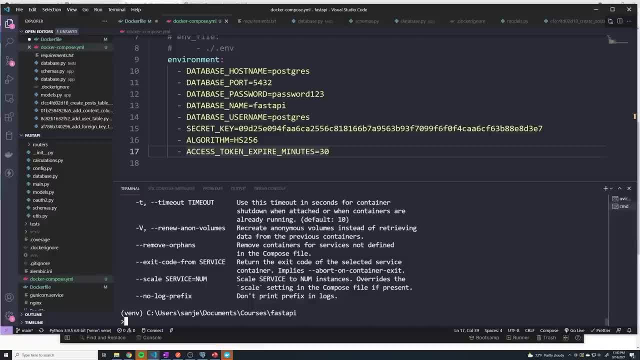 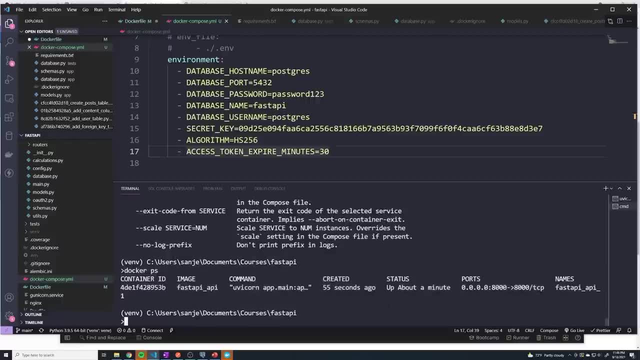 I need you to rebuild it for me, because Docker compose can't detect that. Alright, so now if we do a Docker ps, we can see that it's running now and it didn't crash And we should be able to access it on port 8000.. 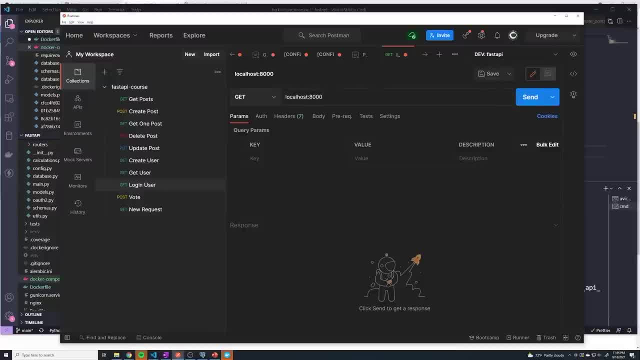 Speaker 1. So if I actually go here and just do localhost 8000, with the get request looks like it's working. Okay. so now that we can actually access our API, which is running in a container, the next thing that I want to do is I want to set up our Postgres database, And you might. 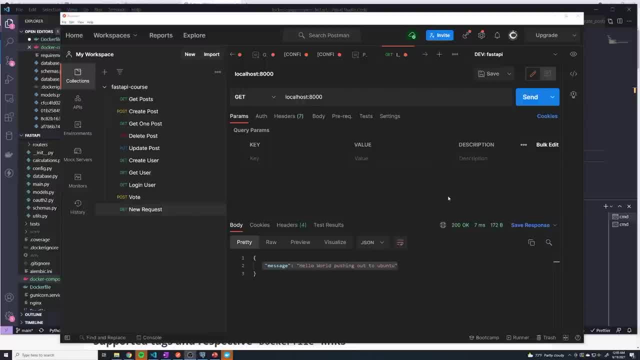 be thinking. well, we already have one installed on a local machine. Why are we setting up another one? Well, couple things. First of all, if we're already Docker rising our environment, it makes sense to set up our Postgres database, especially. 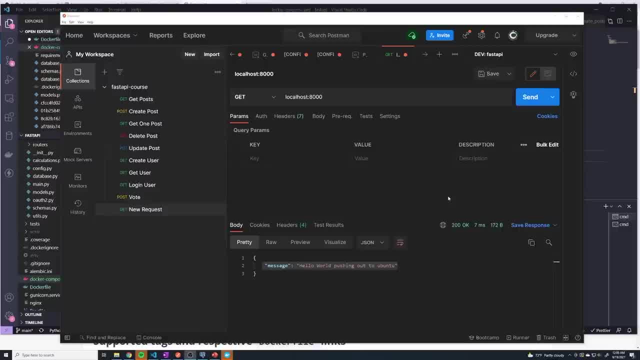 from a development perspective, within a Docker container, because it's so much easier to set up a database in a container than it is to install it on our local machine, because we just spin up a pre built image And that's it. So, even if you don't actually want to, 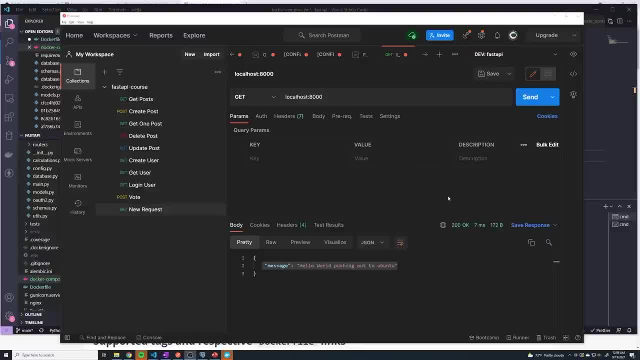 Dockerize your application. from a development perspective, I strongly recommend you make use of Docker containers so that you can spin up a quick database just for testing purposes. But since we already have a Docker based application now, we're going to just 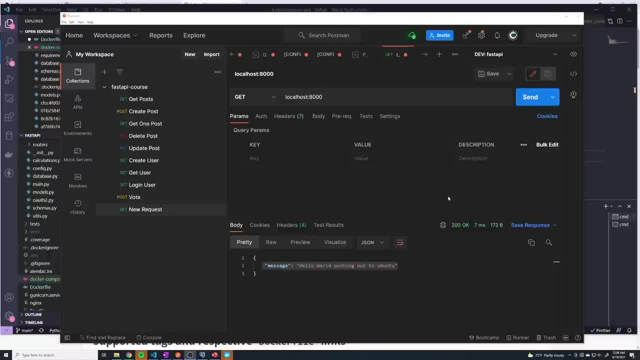 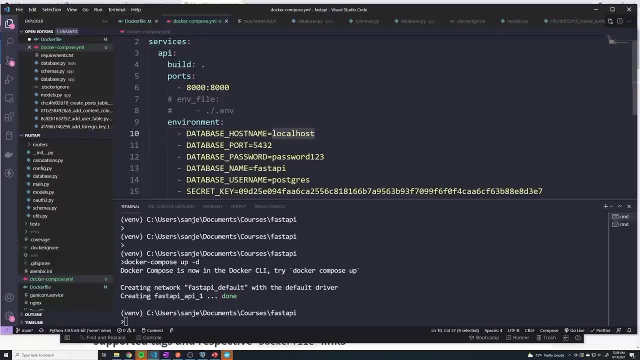 use a Postgres database that's running in a Docker container instead of on our local machine, Because, if we take a look at the environment variables that we pass to our container, we provide a value of localhost, And so localhost means that the container is going to, or the 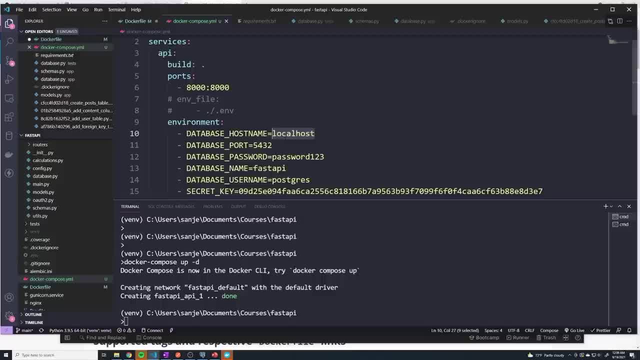 API running in the container is going to try to access a database running locally on that container, which it's not. So let's create a brand new service which, once again, is nothing more than another container for running our Postgres database, And so I'm going to. 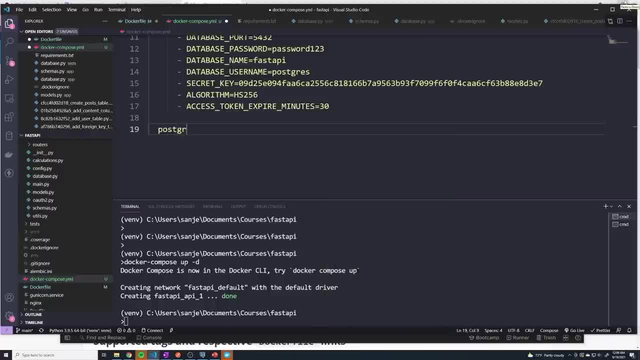 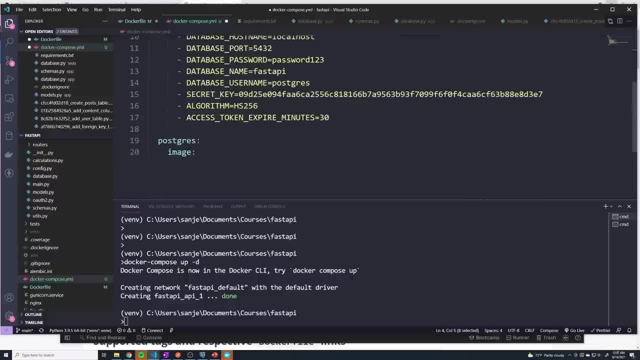 go down here And we're going to create another service called Postgres, And here we're going to provide a image flag right, Because here we did build, because we're building a custom image. Here we're going to use the pre built default Postgres. 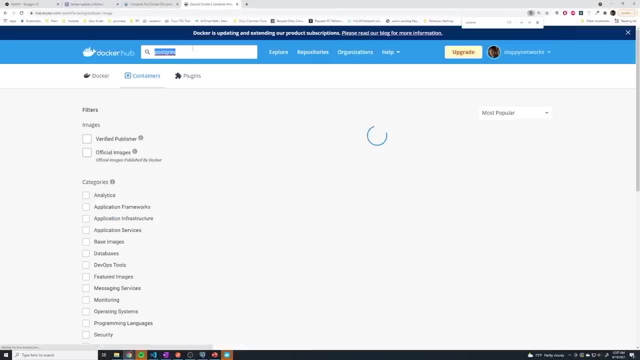 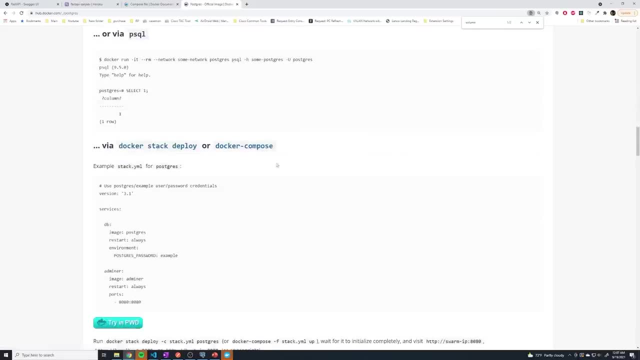 image. So if we go back to Docker hub and search for Postgres, you'll see this is the official Postgres image And this is going to contain all of the documentation for setting up Postgres. But the main thing is there's a couple of environment variables that we have to pass. So first of all, the 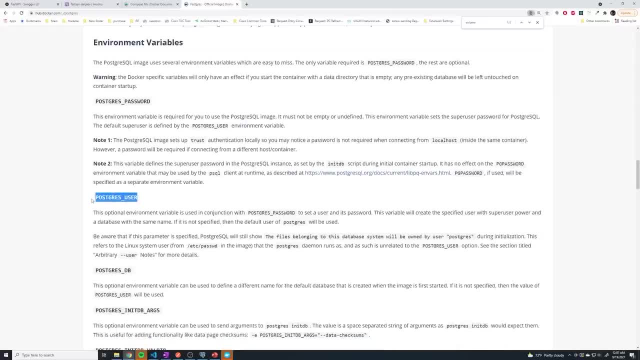 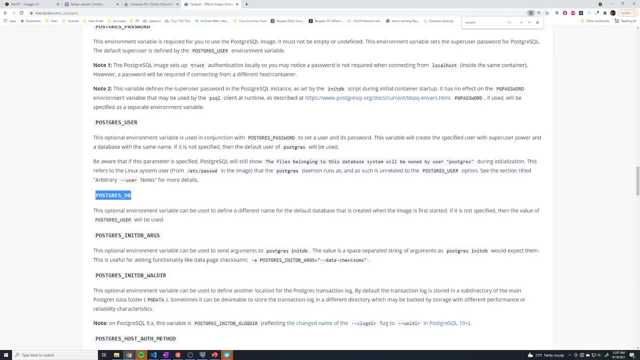 password that's going to be used for our database. we can give an optional Postgres user, but it's going to default to Postgres if we don't provide it. And then we also want to give it a Postgres database name, So we'll call it fast API, like we've been using in our 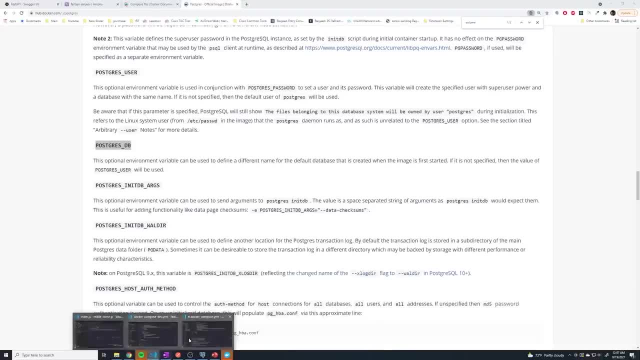 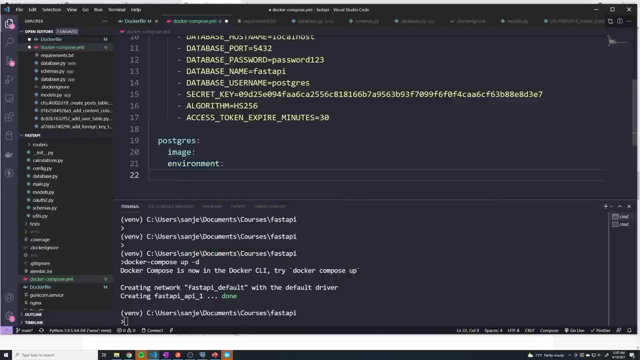 development environment, And that should be all that we have to do for the most part. So here I'll say environment And we'll do Postgres underscore. password equals, and then we can give this anything we want. So password 123.. And then we want Postgres underscore. 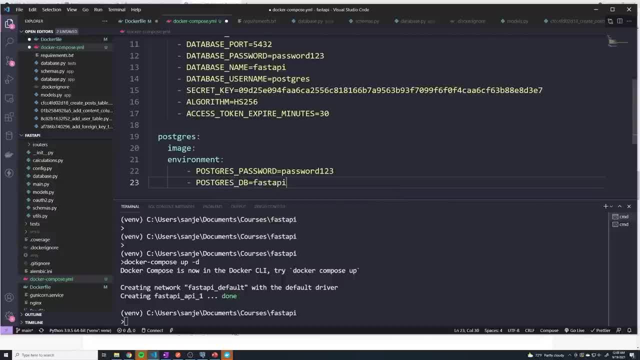 DB. So this is going to be fast API, Alright. the next thing that we want to do is, when it comes to data within a container, that data doesn't persist as soon as the container goes down, Right? So when you delete the container, you lose all of your data, And so from a database. 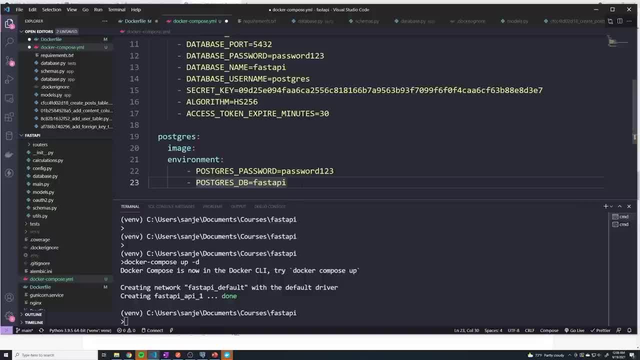 perspective. we don't actually want to lose our data. we want that to persist, even if we kill off the container. So how do we actually save that data? we have to create something that's called a volume, And that's what allows us to save data from a container onto our 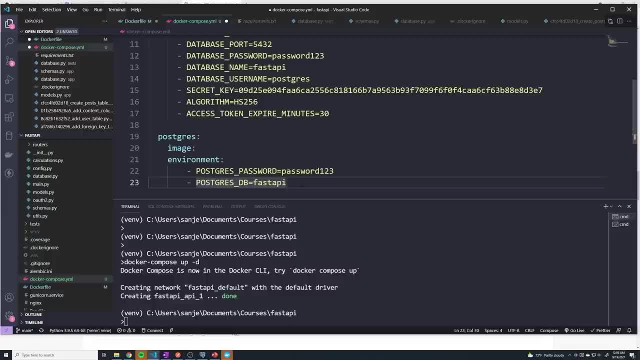 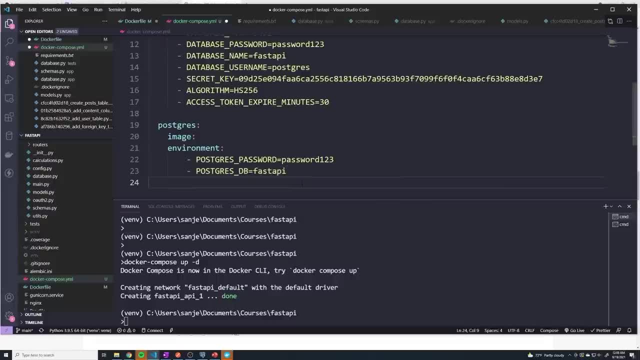 local machine. So if we kill the container we can always spin up a new container and just point it to those files. And there's a couple of different volumes that we can use: our types of volumes and Docker. there's anonymous volumes, named volumes And I think bind mounts is the other. 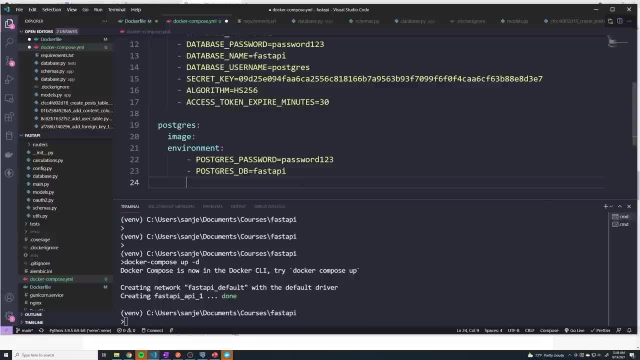 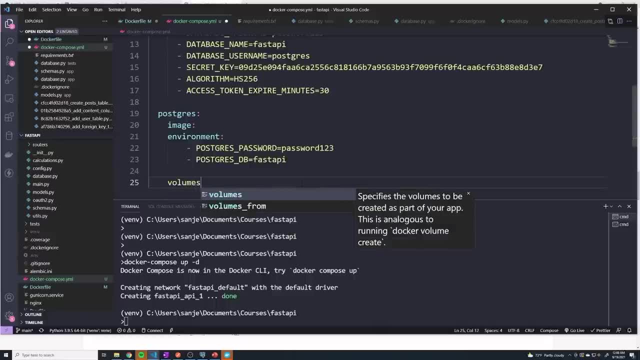 one. we're going to make use of named volumes And so to create a named volume here under the Postgres database section or service, we're going to say volumes And then we say dash and then provide a name for the volume. 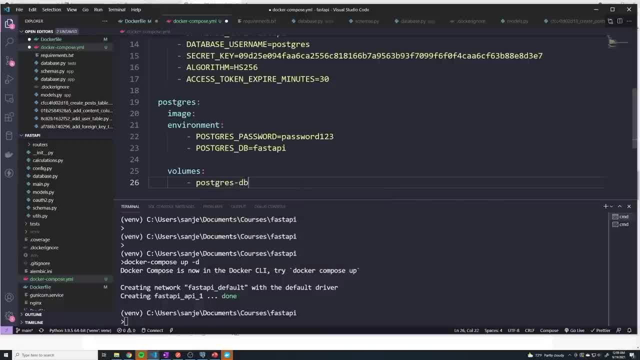 So you call it what you want. I'm going to call this Postgres dash DB Right. and then we have to specify the path in the container that we want to actually save. So what directory do we want to persist on our local machine and the path that the Postgres container or image actually stores all of its? 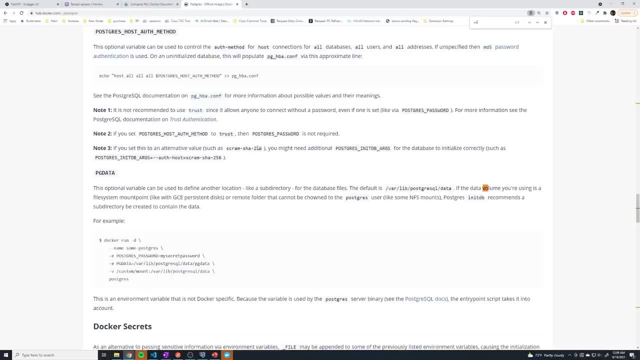 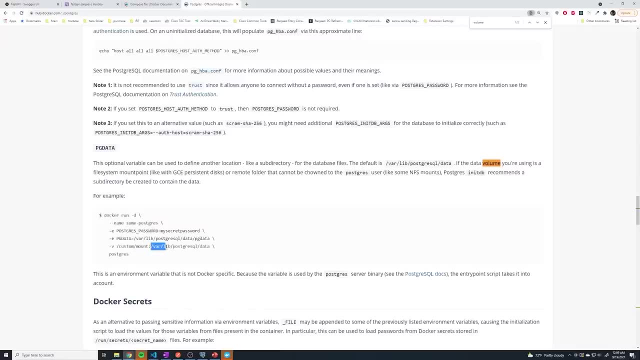 data. we can actually take a look at the documentation to figure this out, If you search for volume, And so right here, this gives us an example And this is going to tell us what we need to know. So we want to save slash bar, slash lib, PostgreSQL, slash data. So that's where it's going. 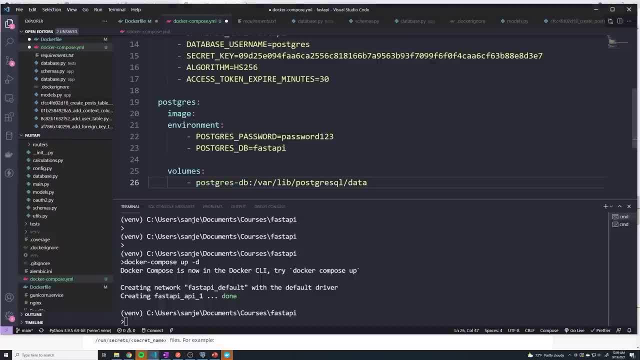 to save all that data. So we'll copy that And, once again, this is the path in the container that Postgres is going to write to, So that's where all of our tables, all of the entries, are going to get stored. So we want to copy that, essentially and save it on our local machine. 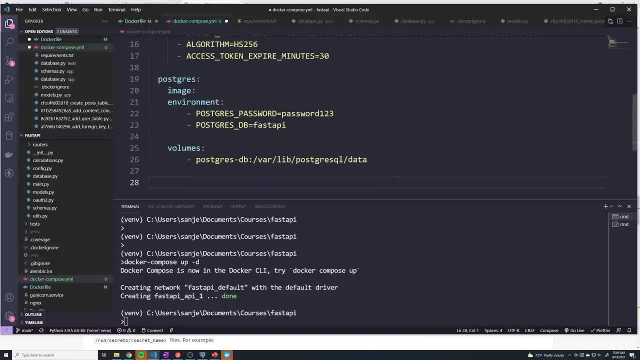 And the last thing that we want to do is, anytime you use named volumes, we have to create another volume section globally, and then just pass the name that we created. So whatever is here, you just put it down here. And the reason we have to do this is because named volumes are. 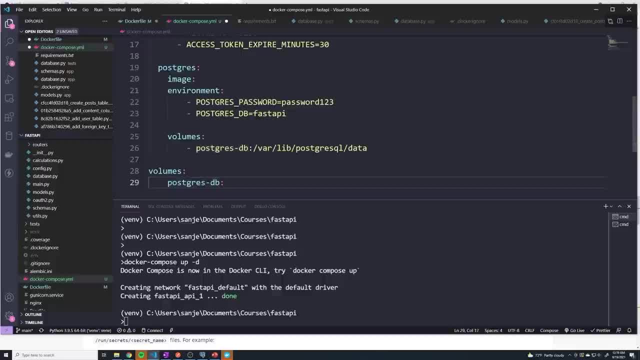 designed to save all that data. So we want to copy that essentially and save it on our local machine So that technically, multiple containers can access them. So you define it down here, first technically and then multiple containers can reference them by just calling that. All right. 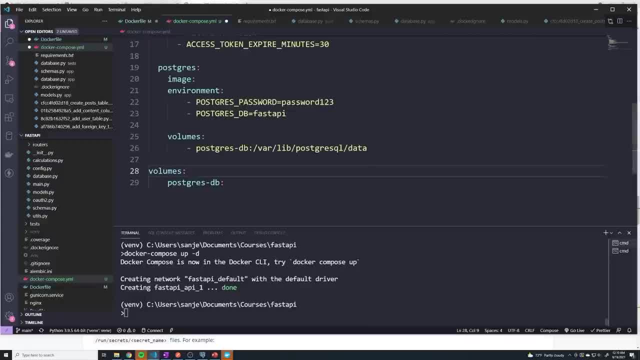 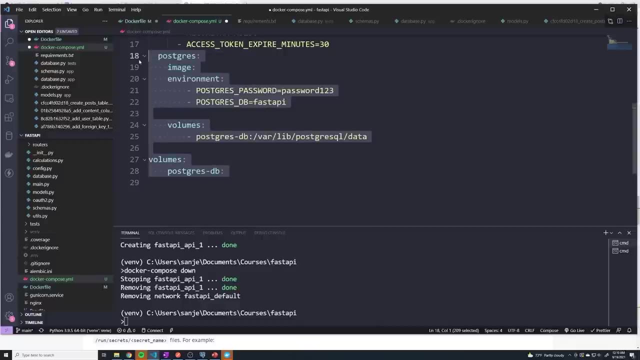 so we've got this setup And actually I realized I left my containers running. So what I'm going to do is I'm going to comment this out for a second, save this, and I'm going to do a Docker compose down That's going to delete everything. then we'll uncomment our Postgres service, Then the next. 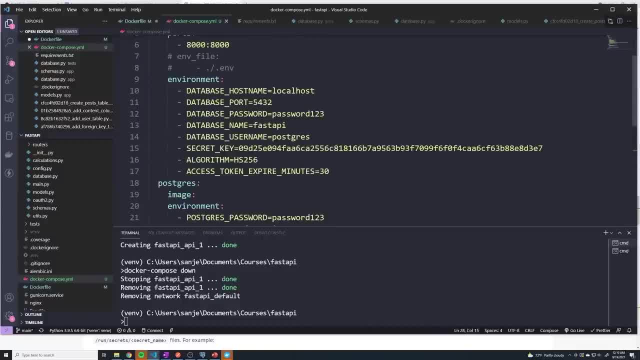 thing that we're going to do is we're going to do a docker compose And then we're going to do a docker compose, And the next thing that we want to do is we have to figure out. you know what is the host name or what's the IP address of our Postgres database, And you know there's a couple of 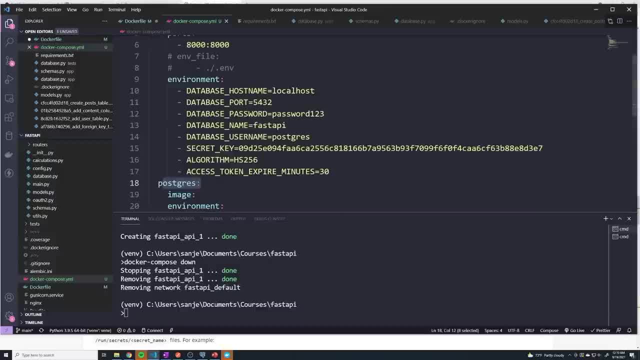 different ways to do that. But what's awesome about Docker is when you use Docker compose, it creates a custom network and a Docker network uses DNS. So we can actually say, to reach the Postgres database instead of like looking for the IP address of that container, we can use DNS And 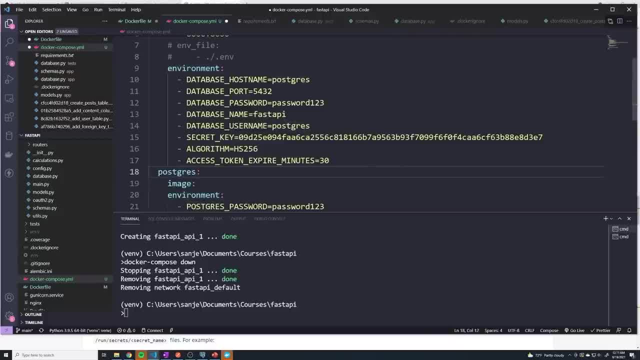 it's automatically going to resolve to our Postgres service. So, whatever our service is called, we can just reference that And this is going to allow this container to know that when you want to talk to the Postgres database, this name here is going to resolve to the IP address of this container. 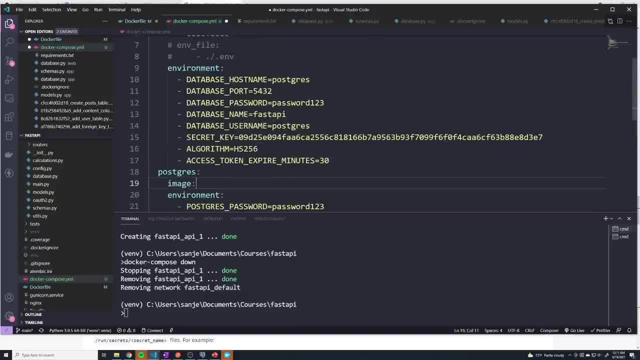 And so networking with Docker within Docker is so simple, because that's all we have to do. And then the rest of the things: the default port, the password, the database name, the database username- those should all be okay, we can just leave as default. And now I can then start this up. 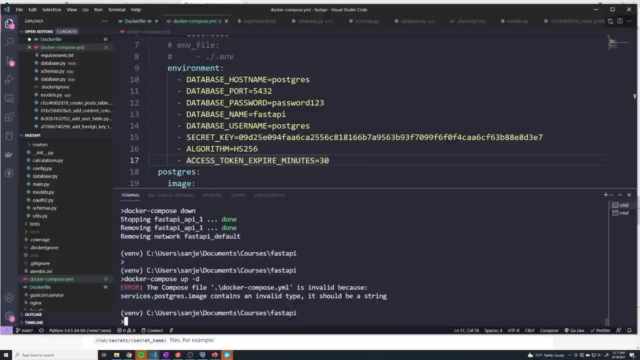 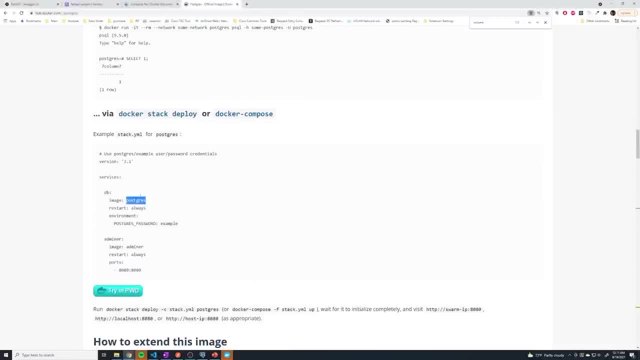 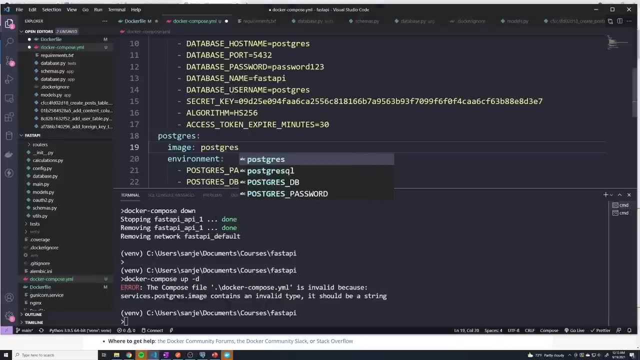 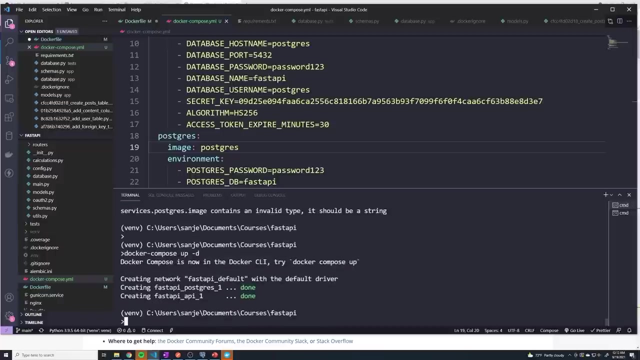 And it looks like image. something's wrong with the image. I forgot to give the image. So what's the image name? It's just Postgres. So that's just whatever this name is. that's all you need. Alright, and so now we can see that it started up both. 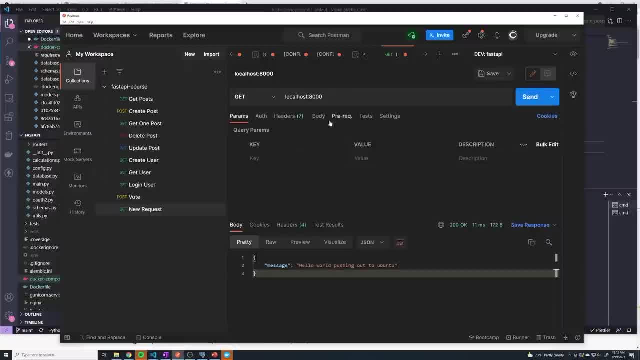 Let's just quickly test our API. So we didn't break anything, So that works. And then let's go to create user. make sure it's point to port 8000.. In this case, and if we create user right, you can see that we have successfully created the user. So it looks like we can now. 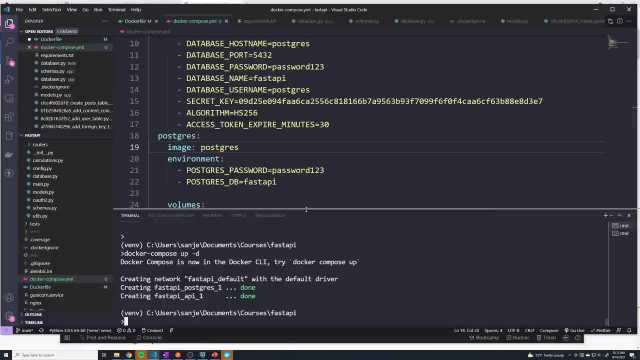 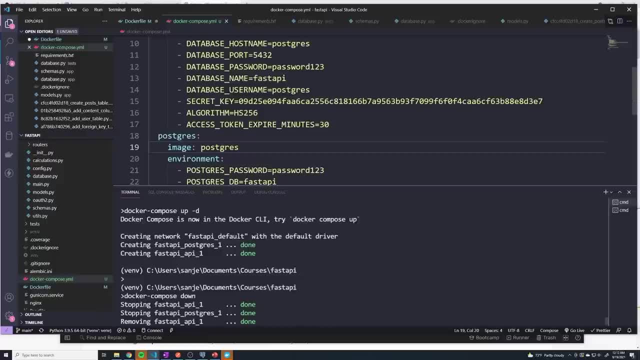 access the database from our fast API container. Now what I'm going to do now is delete everything again. So Docker, compose down, deletes everything, And you can see I'm essentially able to destroy both of my containers with a single command. And that's kind of the power. 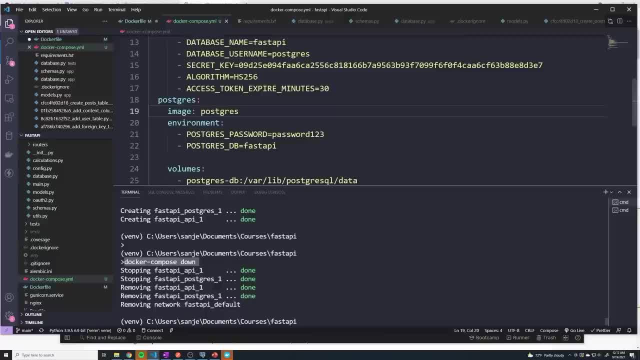 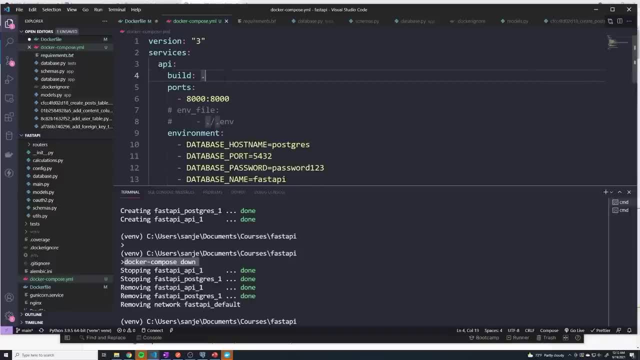 behind Docker compose And ideally we want our Postgres container to start up first, because our API is dependent on the container. So for our API we can pass in another option And I can say depends on- And here we can specify a list of services, in this case just Postgres. 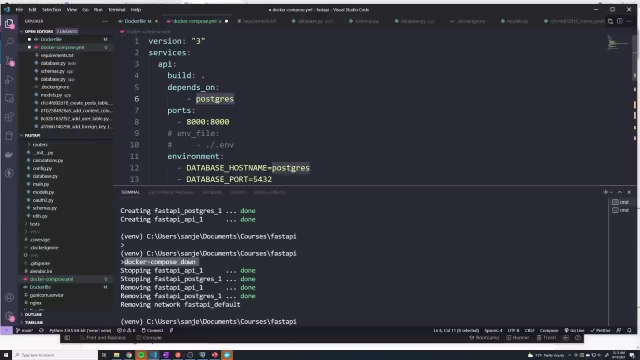 And so this is going to tell Docker: I want you to start the posters container before the API container starts. Now, technically, it's not going to wait for Postgres to actually fully initialize, it'll just start the container. So you still want to put in checks in your code to. 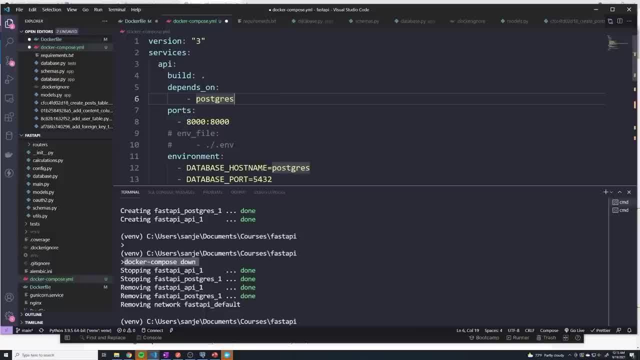 make sure that you know. if you can't access the database because it's not initialized, you want to keep retrying, And so, once again, we can bring this back up with a single command, And if you take a look at the order, you can see that we started up the database first. 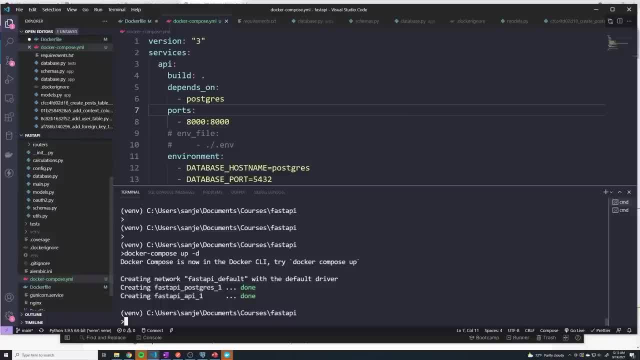 So now you'll always start up your database first and then start up fast API, And then you'll stop fast API first before stopping the database, because we set up the depends on. when it comes to working with Docker containers, we do experience a few extra challenges, especially from a. 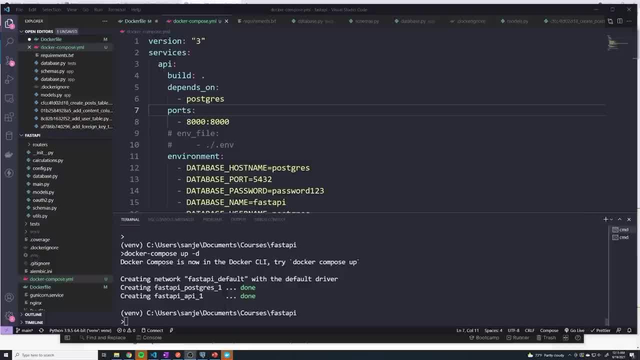 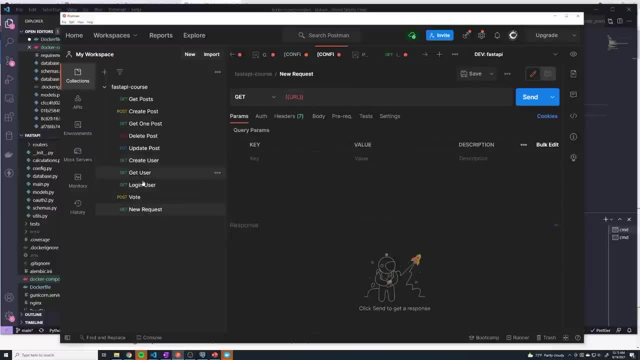 development perspective And I'm going to show you how those challenges actually work, or what those challenges actually are, And if I actually go back to my my test request, wherever, that is where I'm just going to reach the default URL. So if I hit send, you can see it says hello world, pushing out to Ubuntu, right, And that's. 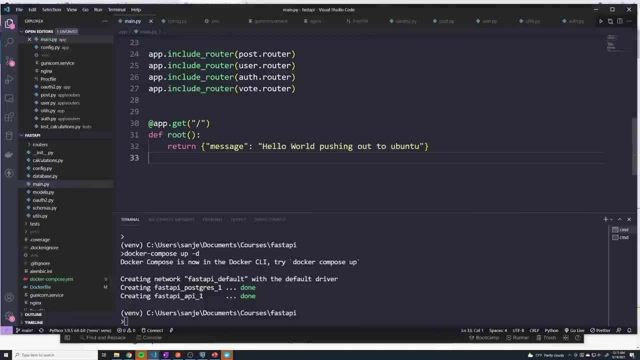 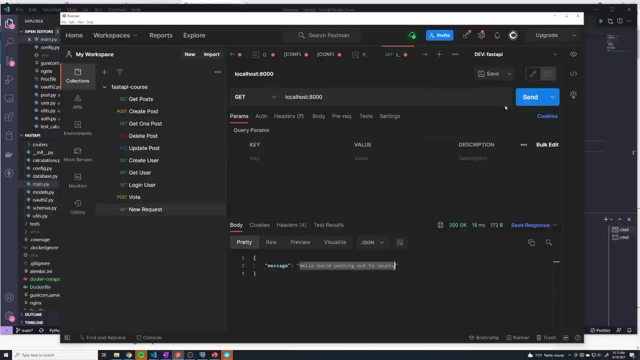 because in my mainpy file is just says: hello world, pushing out to Ubuntu. Now if I save this or change this and then save this, and then I send a request, right, we still get the same response. I don't get the new text that I added. So why is that? Well, there's a couple things that 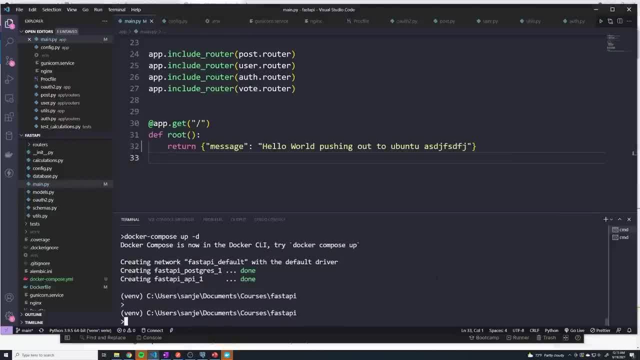 are happening. But the easiest way to figure this out is to actually poke around in your container and figure out what's happening. So I'm going to do a Docker ps And I want to see what the file system of fast API container actually looks like. So to do that, we do Docker exec, dash it. So that's. 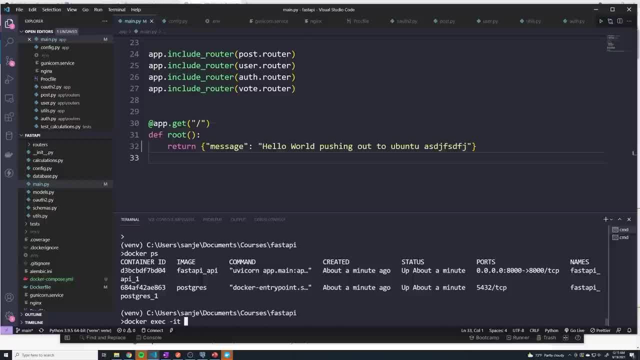 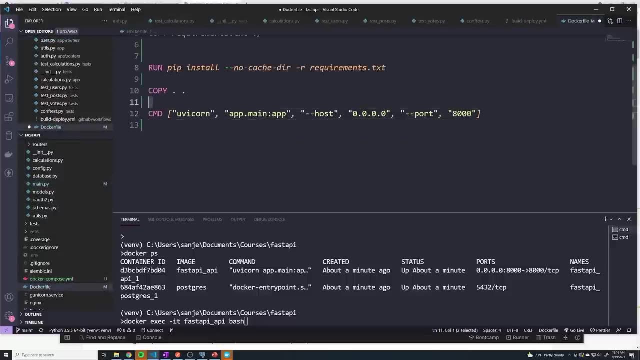 going to enter into interactive mode. we specify the container name and then we type in the word bash. So what we're doing is we're entering interactive mode And we're going to override the default command of the container. So the default command is specified right here from the Docker file. So 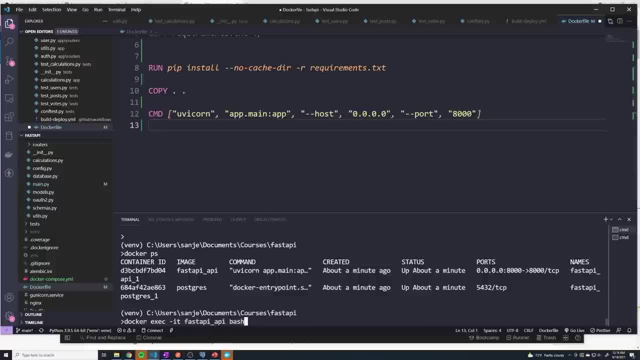 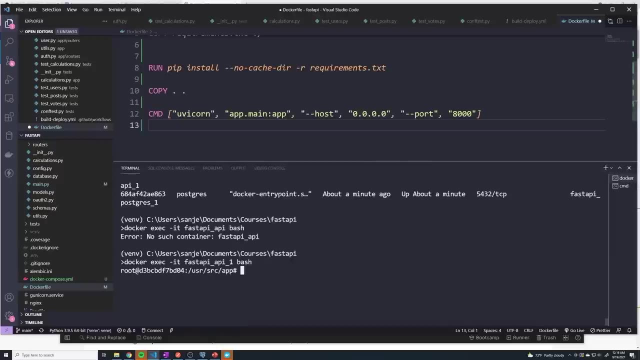 we don't want to run that, we just want to run bash, which is going to allow us to access the file system. That's the image name, So the name of the container is fast API underscore one. So let me add the one. So now you can see that we're. we get a Linux prompt, So we're in the Linux file system. 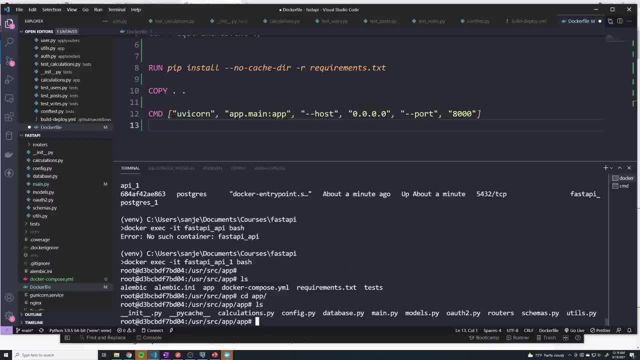 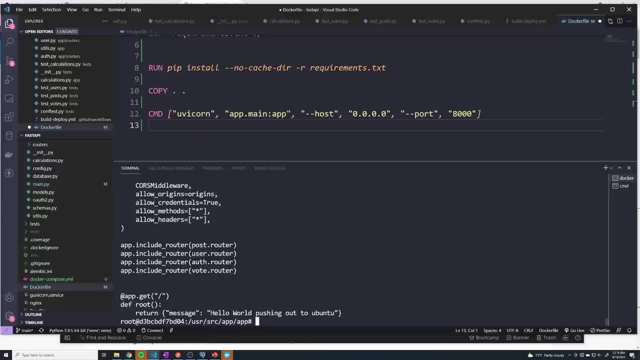 And if I go into app and then go into, if I do cat, which is going to print out the contents of a file, we'll take a look at the mainpy file And you can see that it just says hello, world pushing. 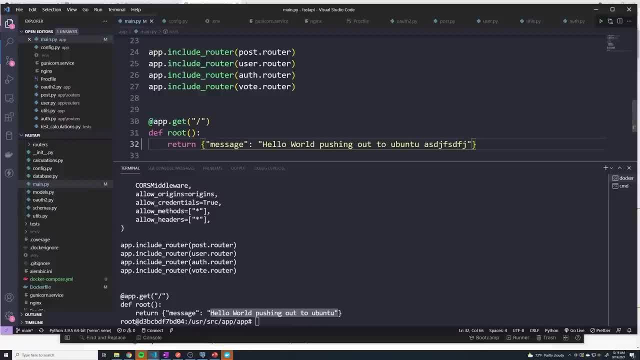 out to Ubuntu. So when I made these changes and added these extra characters, it didn't get pushed out to our container. And if you're trying to figure out why that is, you're going to have to use this script, right? And I don't know why that is. It's pretty obvious, right? Because 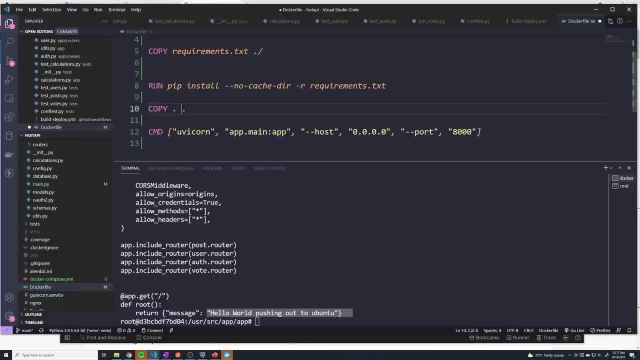 what we did was we created a image which copied all of our code here at that point in time, and then, when we did a Docker compose up, it created the image, And then that was it, Like nothing else changes right afterwards. we went in and change the code, but the image was already created. So 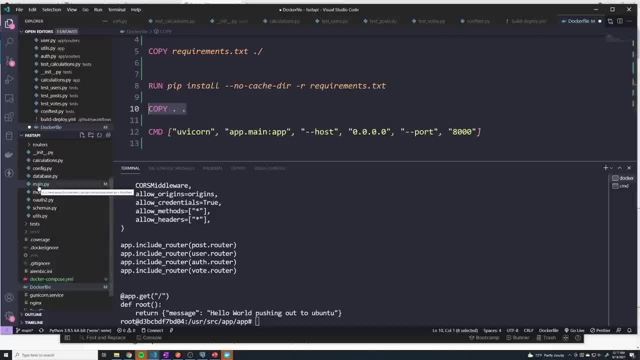 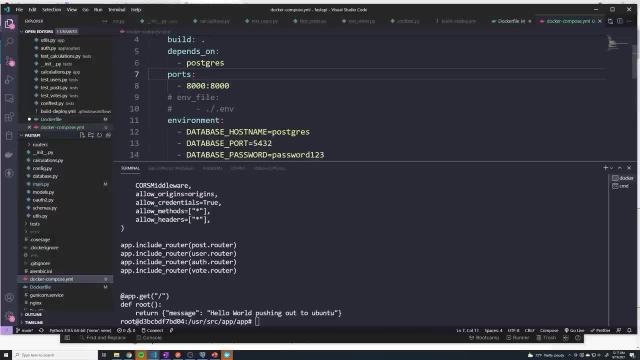 whatever's in the image, nothing changes at that point, So any changes we make will not get copied over to our container case. how do we get around this limitation? Well, what we can do is we can make use of a special volume called bind amount, And a bind mount is a special volume because it allows us to sync. 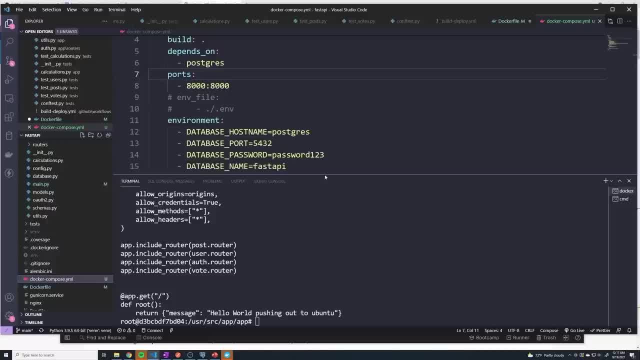 a folder on our local machine with a folder in our container, So this app folder which has all of our application code. what we want to do is we want to sync this folder in our container with this folder here so that if any changes get made here, it's going to get copied. 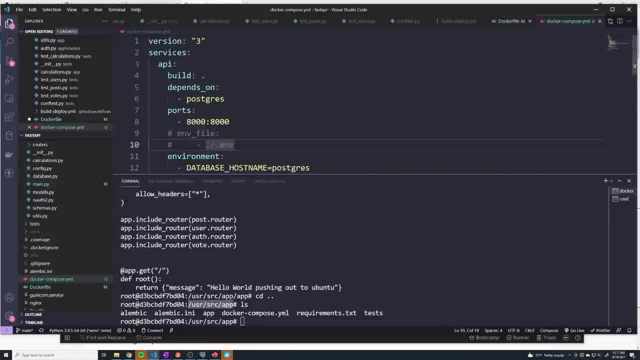 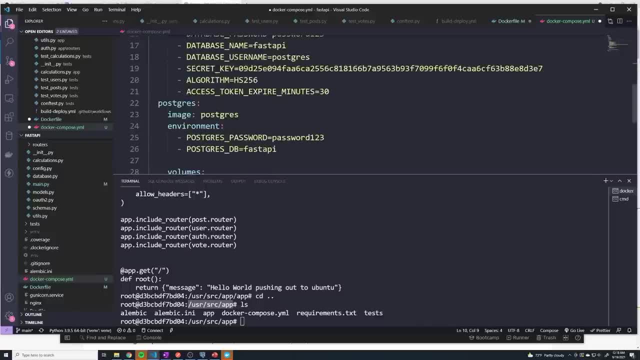 over to our container And so, under volumes in our API, we're going to define a volume here And I'll say volumes Right, just like we did with Postgres. very similar, except we're going to use a different syntax because this is a bind mount. So a bind mount, we have to first provide. 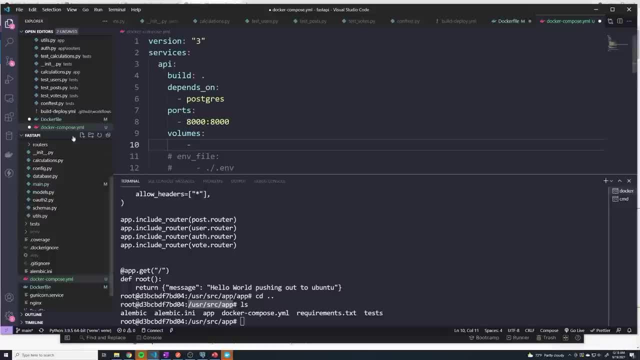 the path of the folder that we want to sync on our local machine. So this is our current directory. So we can just do dot slash for current directory. But if you wanted to sync just one individual folder, maybe like the app folder, then you can do dot slash app up to you. but I'm going to sync everything. 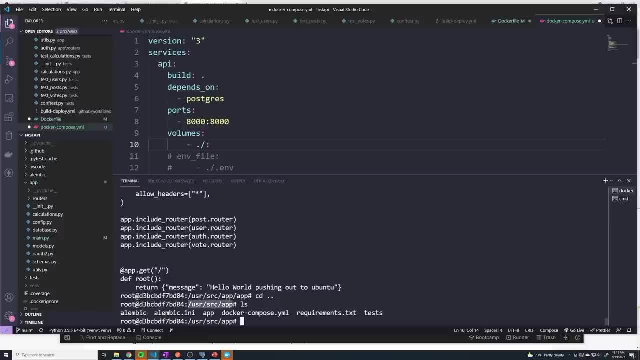 And then we have to specify the path in our Docker container which is going to be this folder right here, And that's going to automatically sync the the two folders. And if you wanted to add some extra security, you can do our. Oh, this means read only. So what this does is this makes it so your 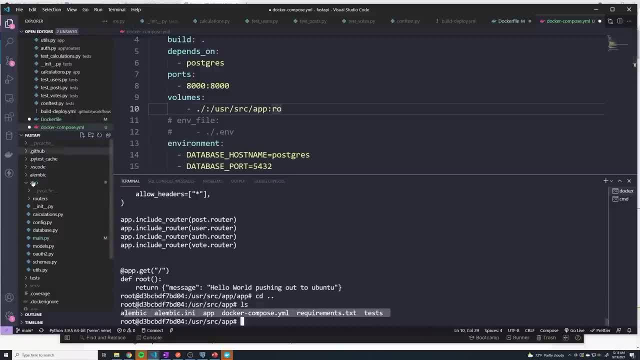 container can't change any of these files, because only we should be changing the files, not the container itself. So this just adds a little bit of extra security, if you wanted to, but it's still technically optional, And let me exit out of here And now we'll do a Docker dash, compose down. 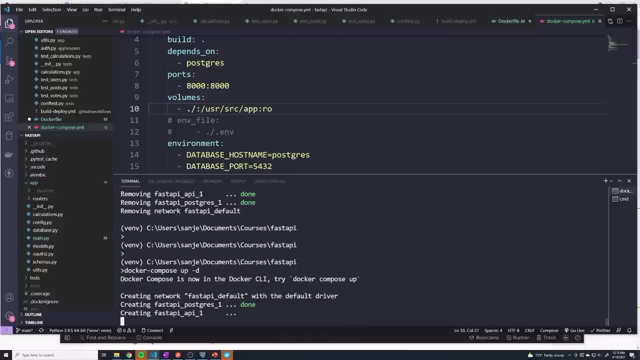 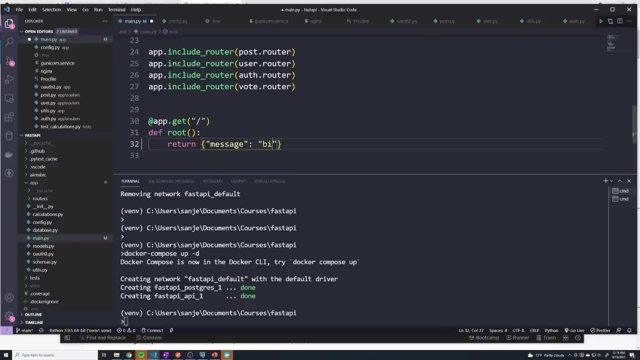 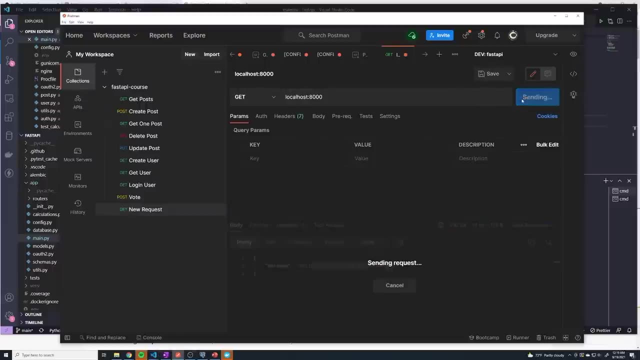 And we'll do a Docker, compose up again. And now let's just change this together altogether. So bind amount works. So if we see that that means everything's working, working, So let's save it. And if I send, we can see that I get the old one now, Right, 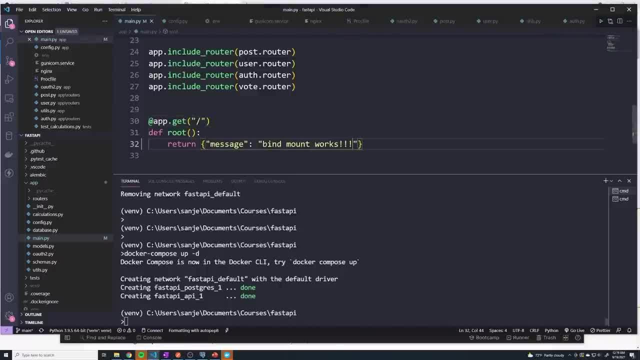 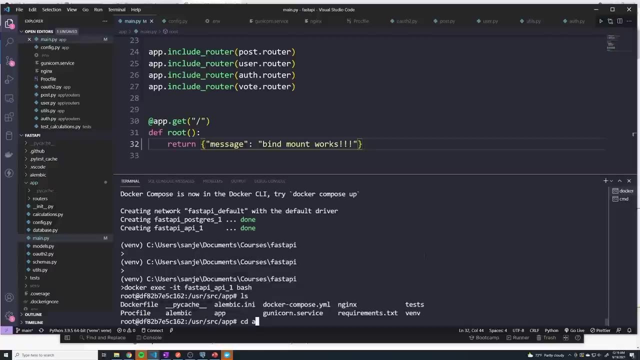 So whatever I changed here doesn't get copied over, So it looks like we didn't fix the issue. So let's actually take a look and see what's happening. And so how do we do that? we'll do the Docker exec command again to go into the file system. Let's go into the app folder. 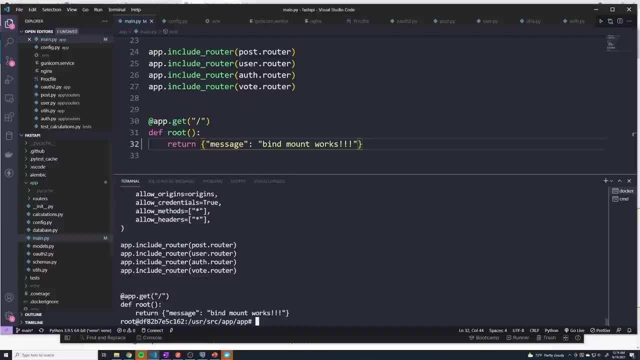 And let's cat that main dot p y file. And this is interesting because it looks like the bind mount did work, because we can see that the code got updated. And if I make another change again, this time let's just add sort of: And if I cat this again, we can see that 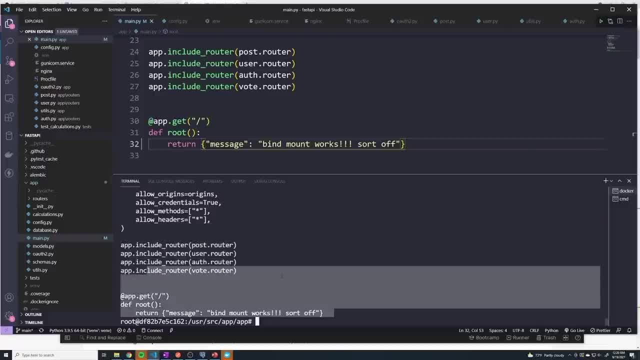 it's in there. So the bind mount is working and it's syncing the code with our local directory and our container. But there's one issue, And if I go back to our local directory and if I go back to our container and if I go, 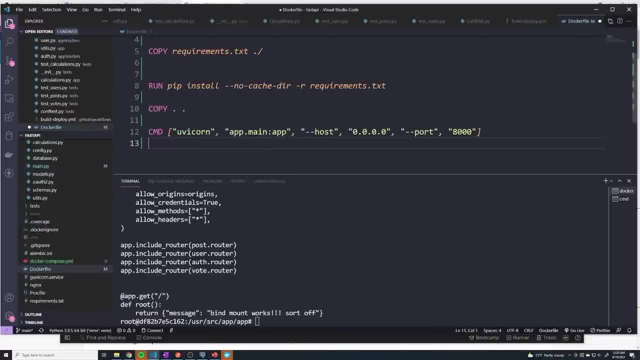 back to my Docker file. you can see that I have my command right here, But this doesn't have the dash, dash, reload flag, which is what we need to restart the application. So anytime we make changes to our code, we need to automatically reload when it detects any changes, so that 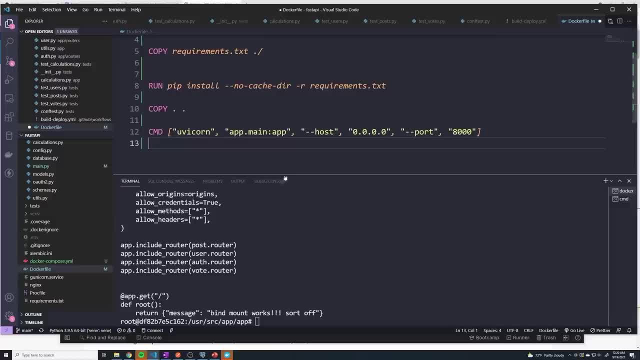 we can actually see the new application, And we didn't provide that in the Docker file, And so that's why it's not working. But this is actually a pretty simple fix. we just add the dash, dash reload flag. So let's tear everything down, And we have a couple options, So I can. 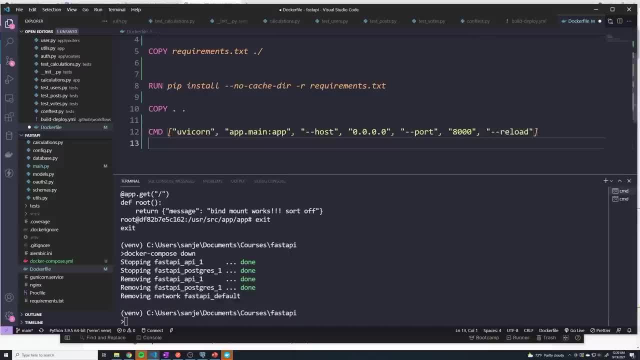 go here and say dash dash reload, And that's would work just fine. But instead of doing that, what I would rather do is I like this default one, because this is the one you technically use in production, because you don't want. you don't want dash dash reload in production, But in our Docker. 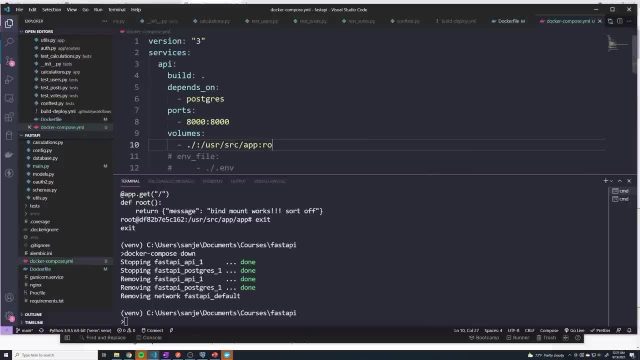 compose file we can actually overwrite it. So we can provide another flag called command. And here we can provide a command to overwrite that from the Docker file. So I'll say Docker, sorry, UV corn app, dot main app. dash, dash host. 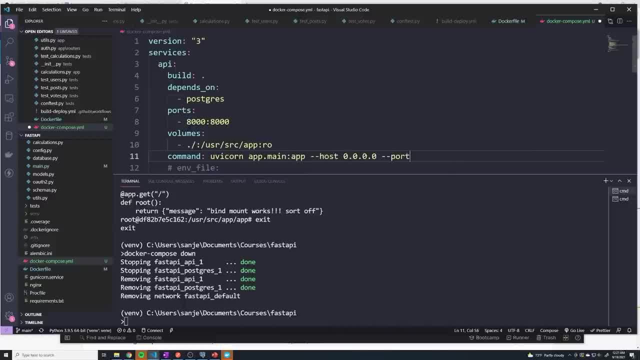 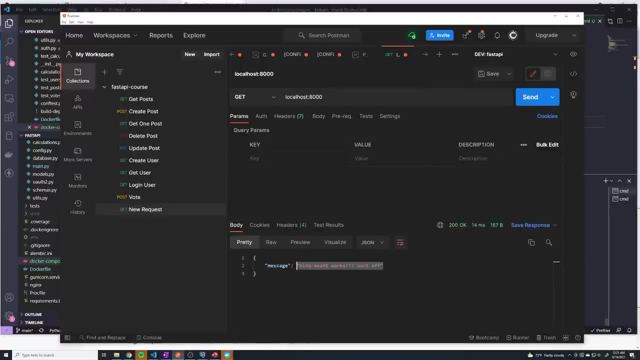 zero, zero zero. dash dash port 8000 dash dash reload. All right, and let's bring this back up. Let's just see what it is currently right now. So we got whatever it is now And let's make a quick. 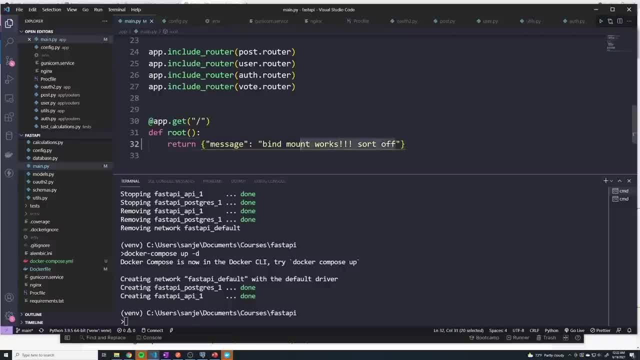 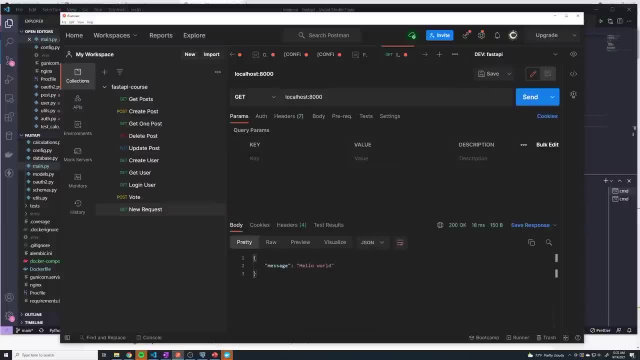 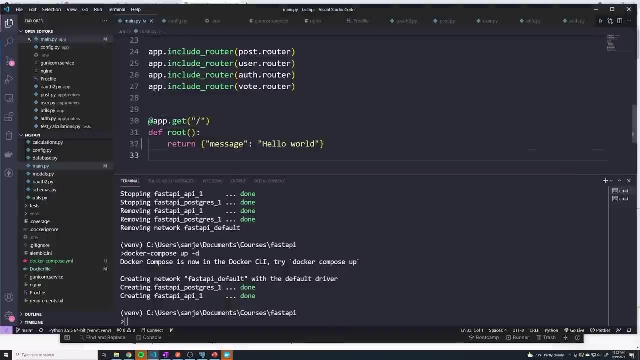 change, And I'll just delete all of this and change this back to Hello world And let's test this out, And we can see that it does successfully update. And so now our bind Mount works and we automatically restart our code, So our development environment more closely matches up with what was what we had. 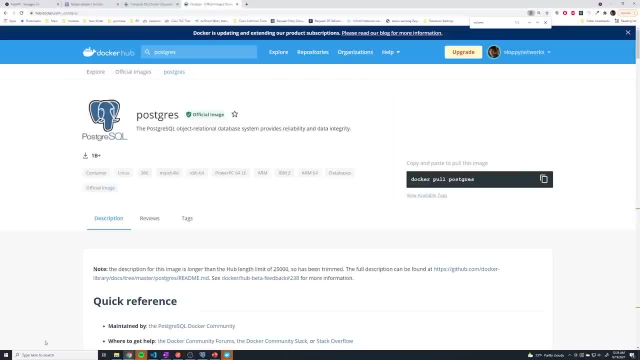 before, before we moved to Docker. Okay, so if you haven't already done so, go ahead and create an account on Docker Hub. It's a free account. So just go ahead and go ahead and create an account on Docker hub. It's a free account- And then I'm going to go ahead and try to import questions in it. And then I'm going to hit OK, so that's going to send these in there in the final version. Okay, there we go. So there we go. So that's the basic version of what we're going to do. So that's a free account. 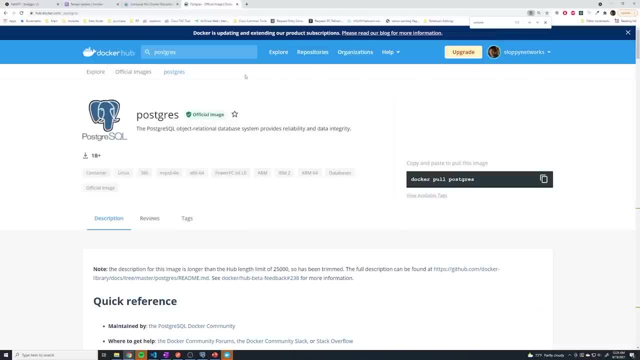 It's a free account, But I want to show you guys how we can set up a repository on Docker hub so that we can actually store our images here, And so Docker hub is kind of like the, the Docker equivalent of GitHub, where it's kind 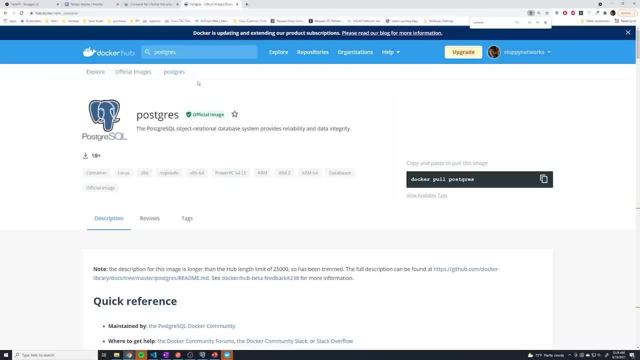 of acting as a repository, But instead of a repository for our code, it's a repository for our images, So we can upload our images. anytime we make a new image, we can actually upload it, so that we can track changes to our images over time. 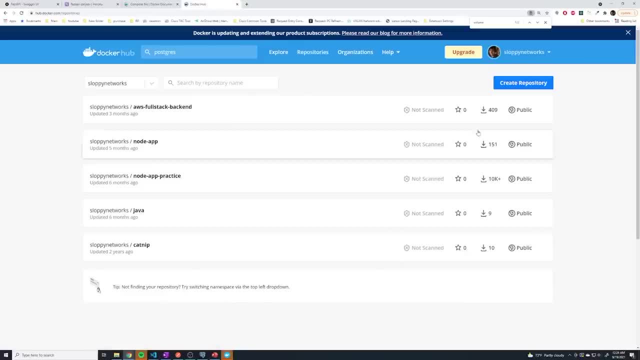 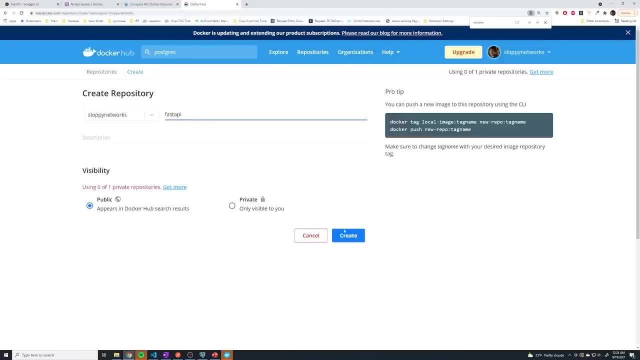 So make an account And then we want to go into repositories And we want to select, Create repository and then give this a name. it doesn't really matter what you want to call it, I'm just gonna call it fast API. And then we're going to do public, because you only get one private repository. 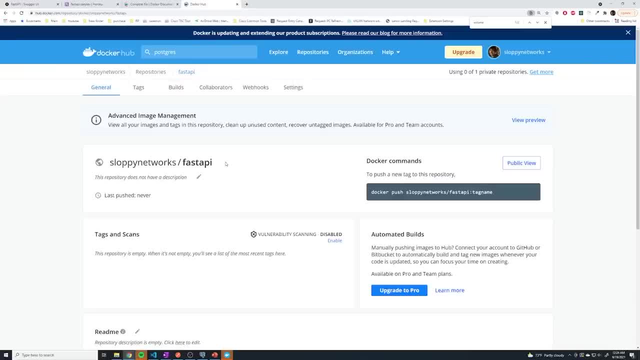 And so now we have a private repository. it's a public repository, And so this is the URL to the repository, which is going to be your username. this is my username, And then this is the name that I gave it so fast: API. 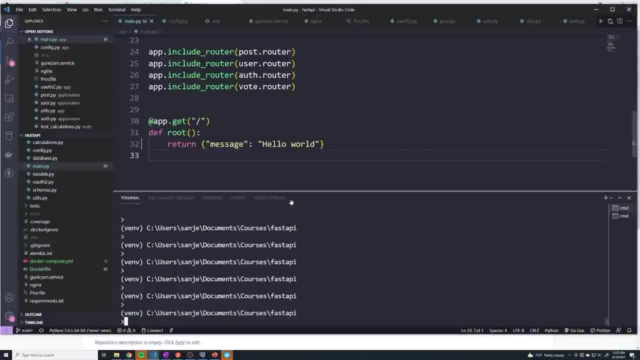 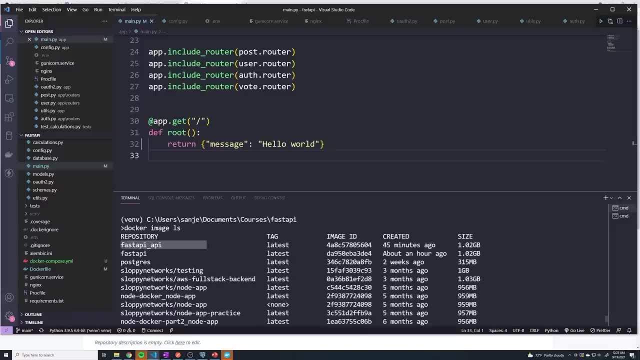 And so now what I want to do is: I have an image Right. If I do Docker image LS, we could see that I have my fast API underscore, API. this is going to be the image that I want, And so how do I actually upload this image to to Docker Hub? 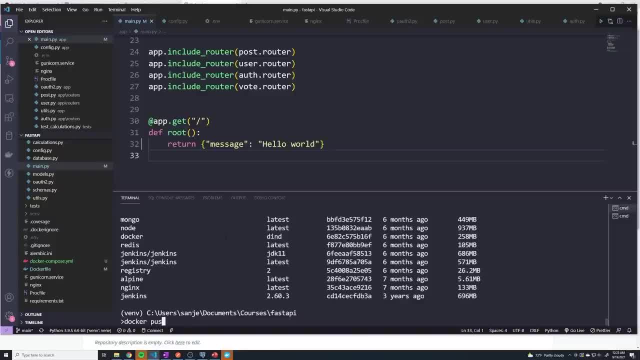 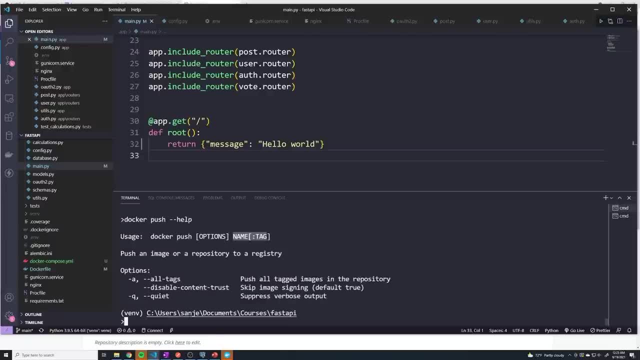 Well, there's a command called Docker push, Right? So if I do a Docker push, dash, dash, help. you just pass in Docker push and then the name of the image. So let's try doing that. We'll do Docker push. 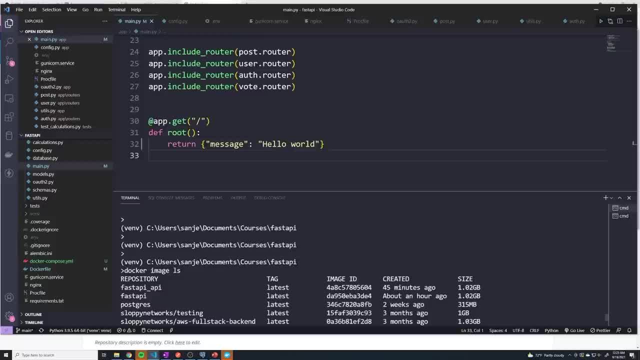 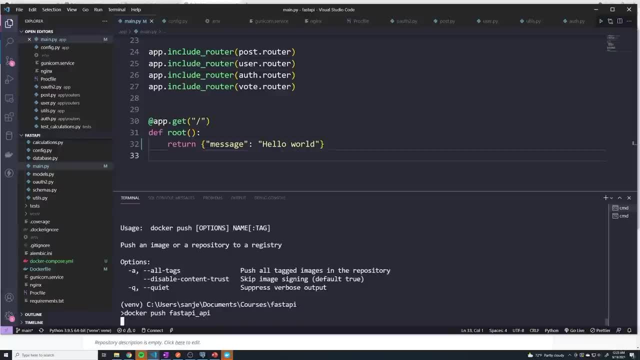 And then the name of the image, which, remember, yours, is going to be a little bit different because it's going to be based off of your, your folder- Let's try this. And it says: requested access to resource is denied. So the first thing that we have to do is we actually have to do a Docker login, so we 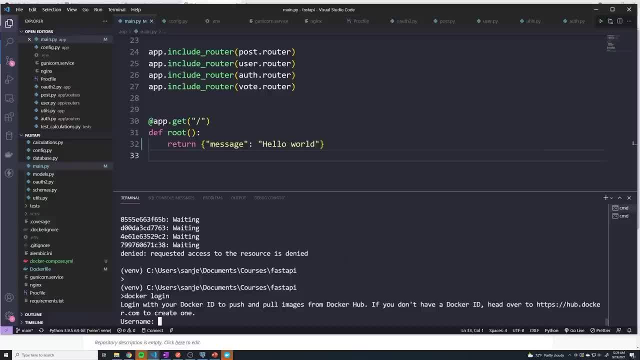 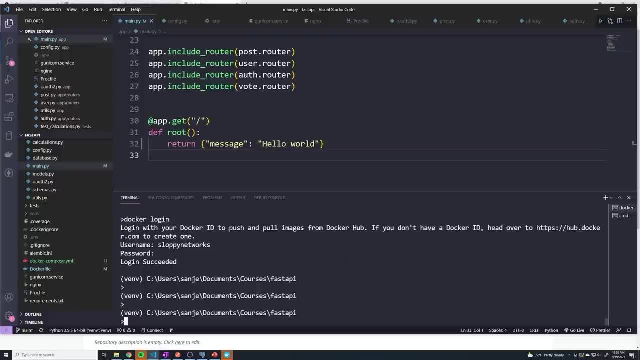 have to log into our account. So you do Docker login here. it's gonna ask for your credentials. So we'll do sloppy networks, in this case for me, and then it's gonna be whatever it is for you guys. And then now let's try to push it again. 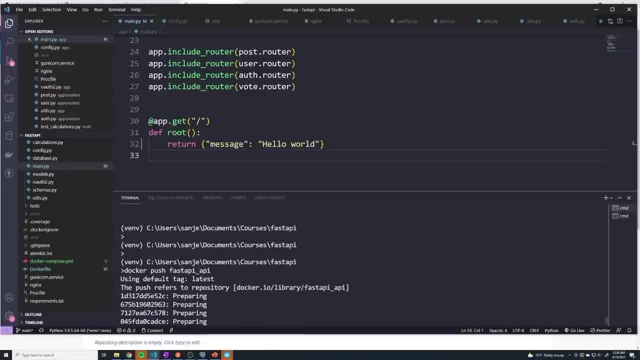 And once again we get: a access to resource is denied. So what exactly is happening here? Well, when we want to push up a image, right, there's a very specific naming convention that we have to use. Right, we have to name it exactly like this: sloppy networks- slash fast API. 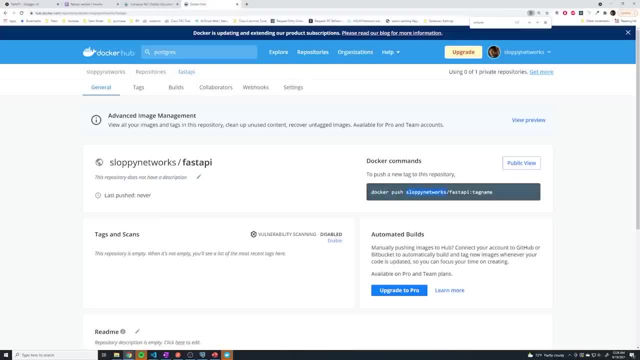 And we even see an example right here. So you do, Docker, push the name of your email or your account name, then the name of your specific repository and then you can give it an optional tag name. So what we got to do is we got to rename our image. 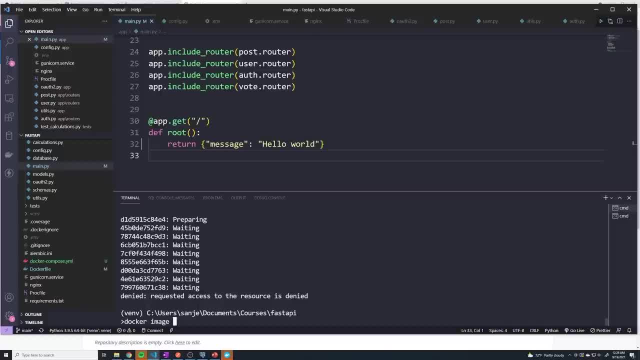 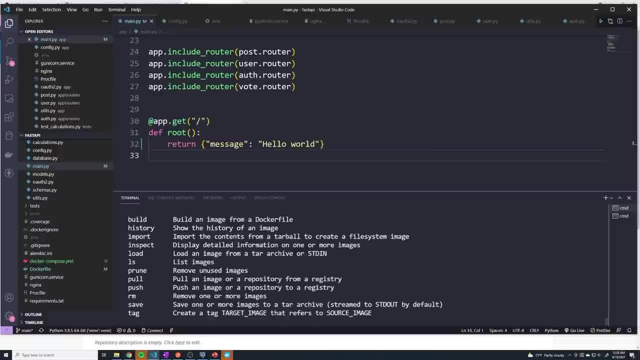 So how do we do that? I think it's Docker image, I think. well, let's do dash, dash help, just to see if we can figure it out. We want tag, So this essentially copies an image and renames it for you. 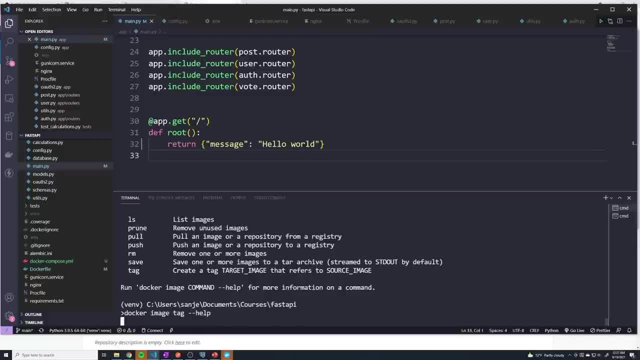 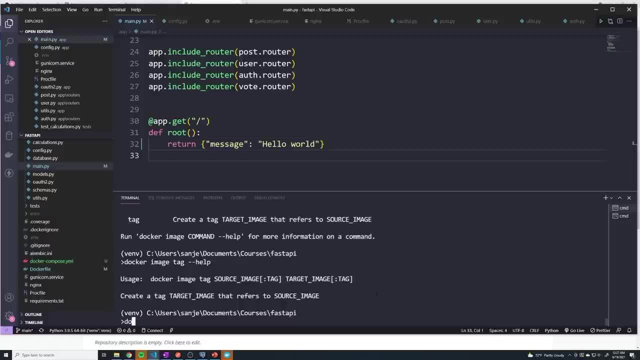 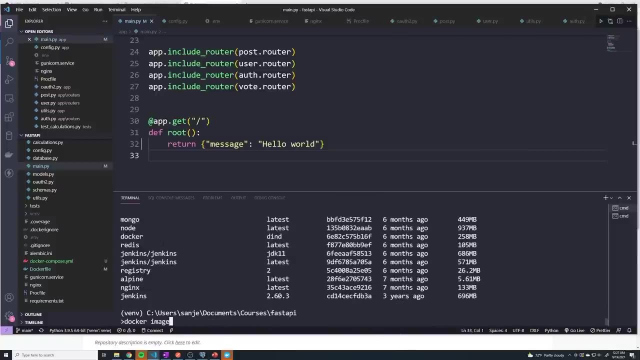 So let's do Docker image tag, dash, dash, help. And here we just provide the, the source image and then the target image. So what is my image called? again, it's going to be this one right here- And we just do Docker image tag, then the image that we want to rename, and then we 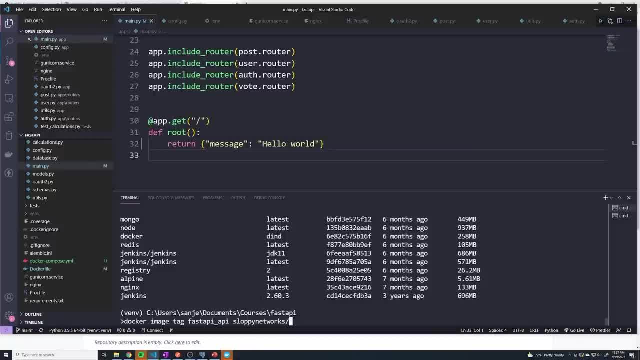 give it the new name, which has to be your account slash, then the repository and then you have an optional- you know- tag. the default is just going to be latest, So I'm just going to leave it without a tag. 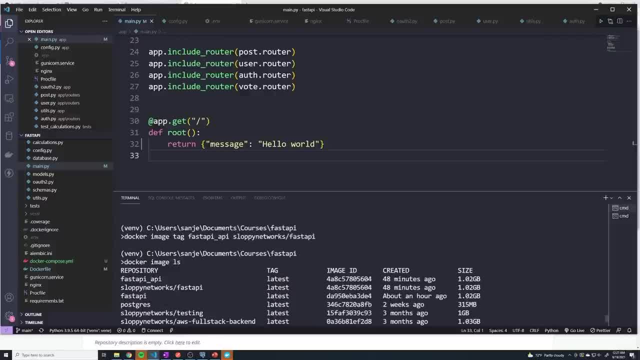 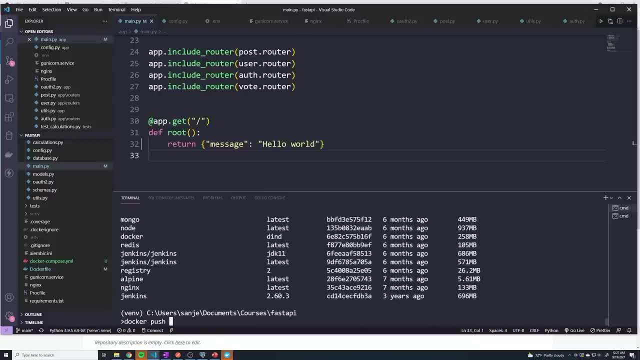 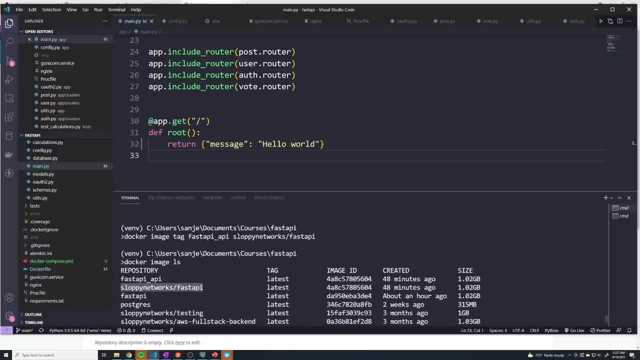 So I do that, And if I do a Docker image LS, we should see the new one right here, And so now I can do a Docker push. It looks like I didn't copy that, So let's try this one more time. 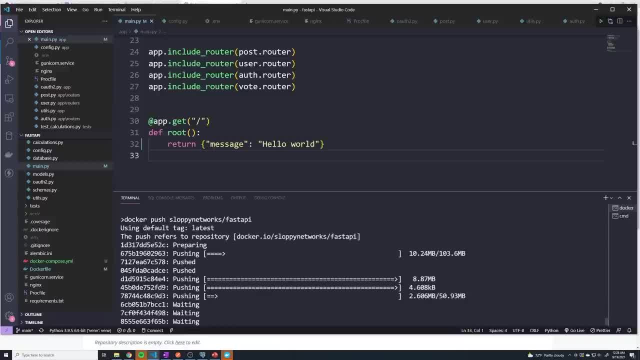 And now it looks like it's pushing something. So let's give this a minute or two And then, once it's done, let's take a look to see if we have successfully pushed it to our repository. Alright, so it looks like it's successfully pushed. 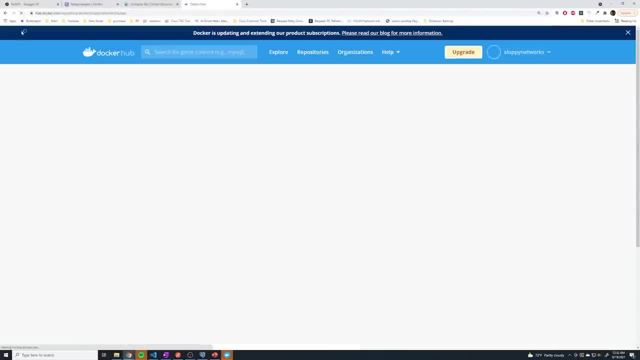 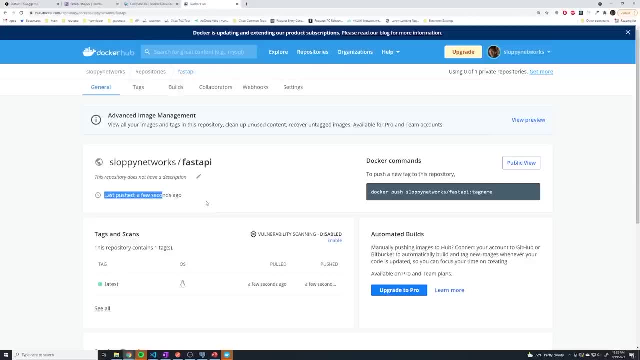 So now, if I go back to my Docker hub page and do a refresh, we can see that last pushed was a few seconds ago. So now we've successfully pushed it to our Docker hub. And so you know, if we set up an actual production Docker environment, we could just pull the. 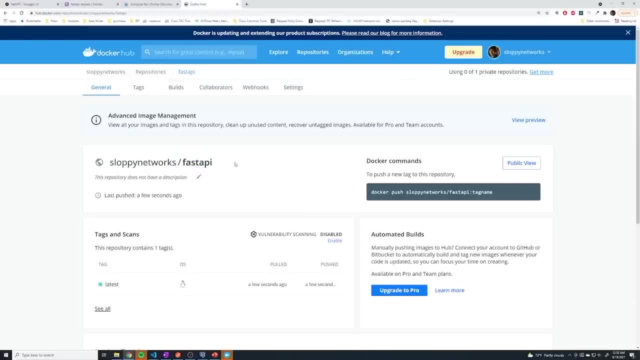 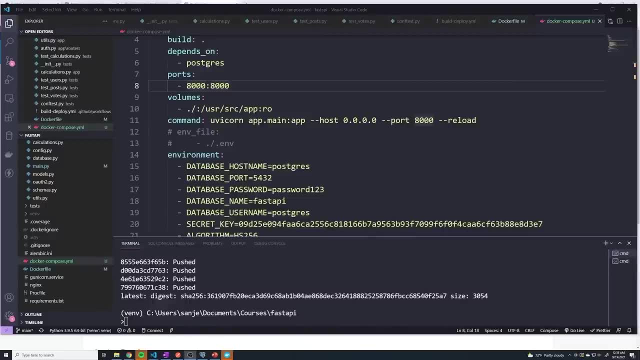 image from this specific URL or this specific repository. Now, before we wrap up the Docker section of this course, there's one last thing that I want to show you guys, And that is that, if you take a look at what we have right now, we have a identical clone. 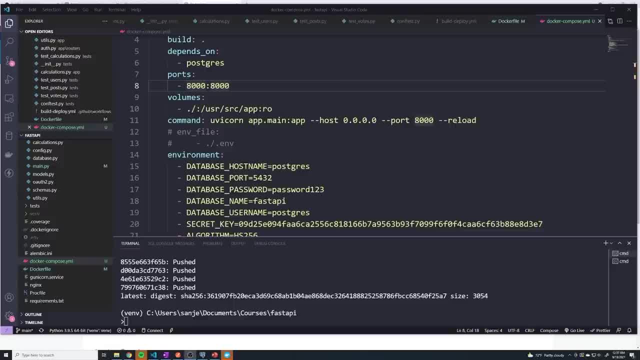 of our previous development environment, but we're now developing within a Docker container, So our Docker container environment is a exact clone of our previous development environment. The issue is: is that you know when we move to production, assuming that you're using 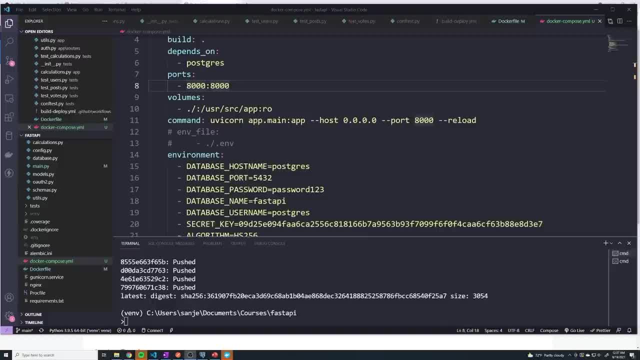 Docker in production, which is kind of the main idea behind Docker is that your development environment and your production environment are almost exactly the same because you're using the same exact Docker images and containers. But if we try to use this Docker component Post file in production, there's going to be a whole bunch of issues. 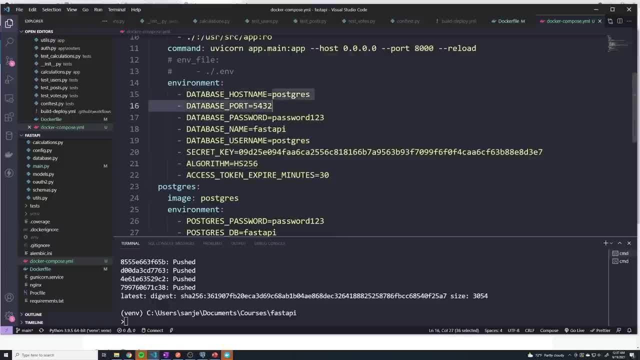 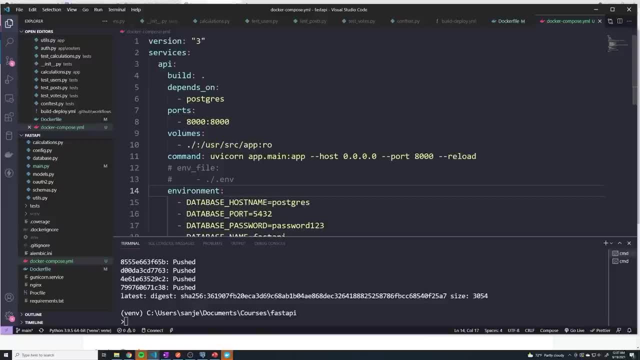 First of all, obviously these environment variables would need to change and we can't hard code them. We wouldn't want the dash dash reload flag, And you certainly don't want to bind mount, because the code shouldn't be changing, And then the ports that we use could also potentially be different. 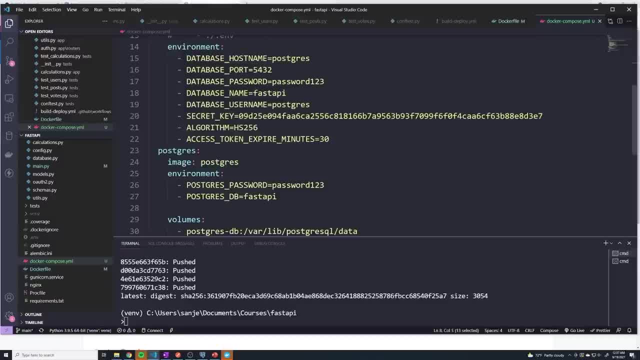 So even though Docker, or so even though the Docker environments from our production environment should be roughly similar, there are going to be some differences, And so we need to account for that, And so what I like to do is I actually like to create two different Docker compose files. 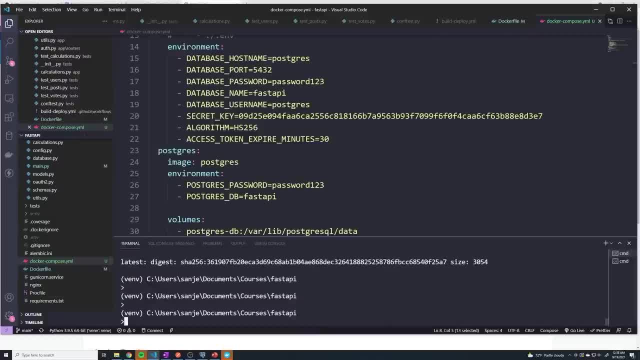 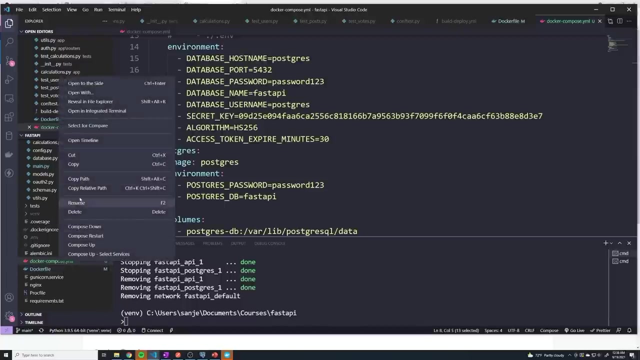 one for development and one for production. So that's what we're going to do, But first of all, let's do a Docker compose, dash down that we can just tear everything down for a second, And once that's down, I'm going to copy this: 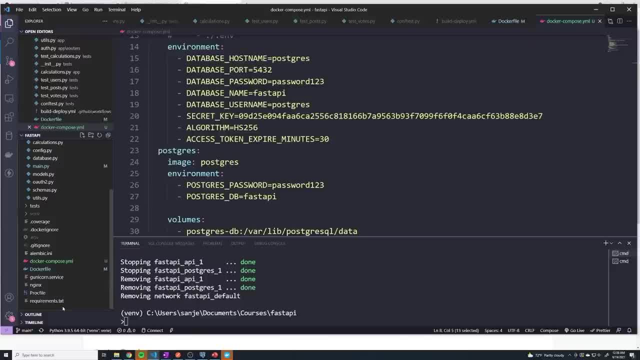 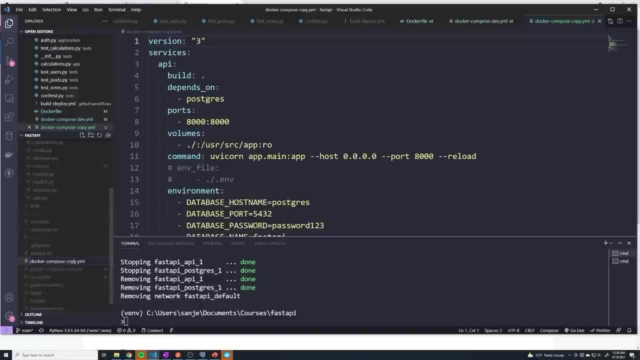 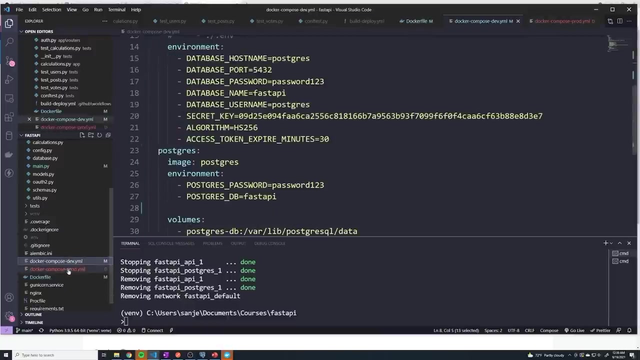 And paste it, And we're going to rename these files. So this one is going to be called Docker compose dash dev. So this is going to represent our development environment And this one is going to represent our prod environment. Alright, so we've got our dev and our prod environment. the dev doesn't need to change. 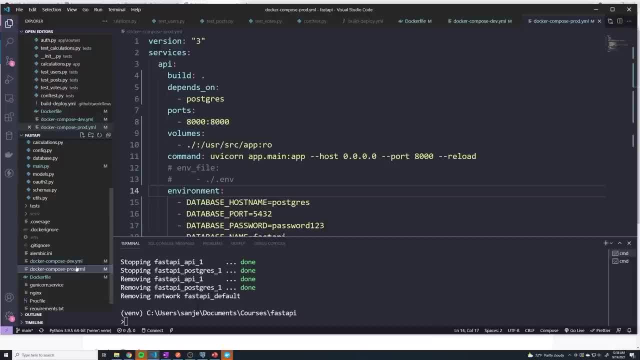 because we had already set that up for development environment. The production one is going to change a little bit. So first of all, the command. right, we don't want the dash dash reload, so we could specify the exact command we want, which is the one without the dash dash reload. 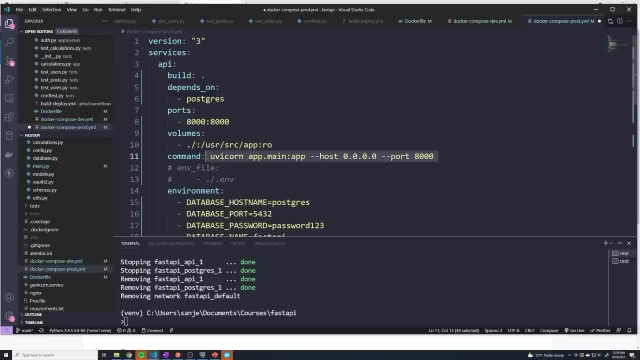 And that should be all that we need. However, keep in mind, this is the default command from the Docker file, right? So we could technically just remove this or just comment it out, And so I'm just going to comment it out in this case. 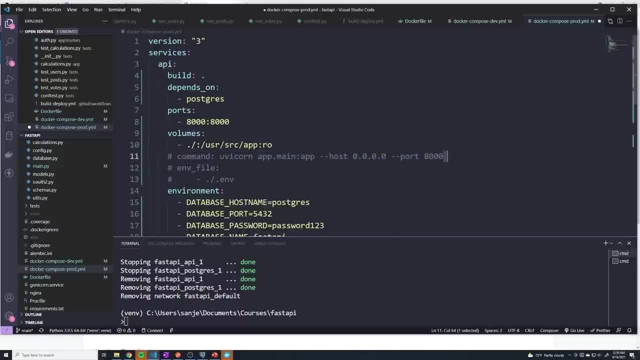 But if you wanted a specific custom command for production, you can just provide that here, And the whole idea is that this file is going to represent all the changes for our production environment, Then maybe we want- instead of listening on port 8000, we want port 80, so that we can. 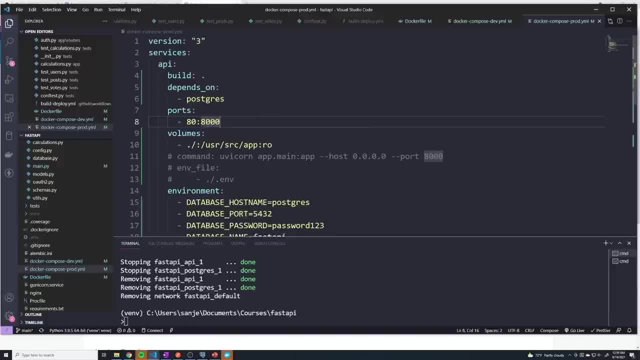 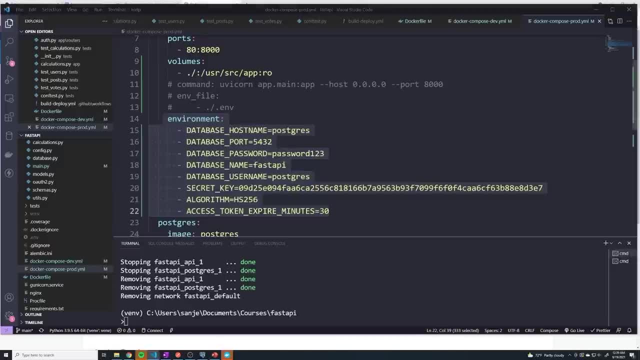 use our web browser, Most of the things can stay the same. the environment variables definitely need to change, And so, with a production environment, we, first of all, we're not going to hard code the values. we usually want to grab. these. 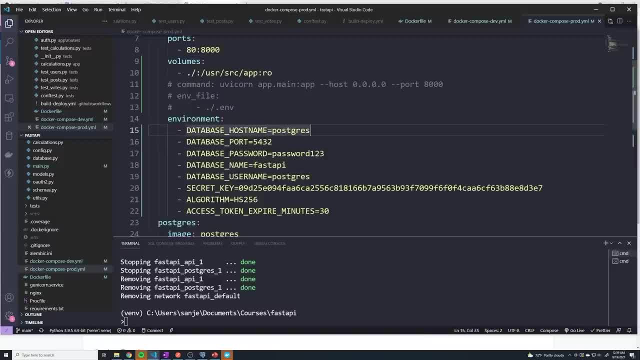 These values from the environment variable set on the host machine. So instead of actually hard coding these in, instead we can reference environment variables. So to reference an environment variable, what we do is we do dollar curly braces and then the name of the environment variable. 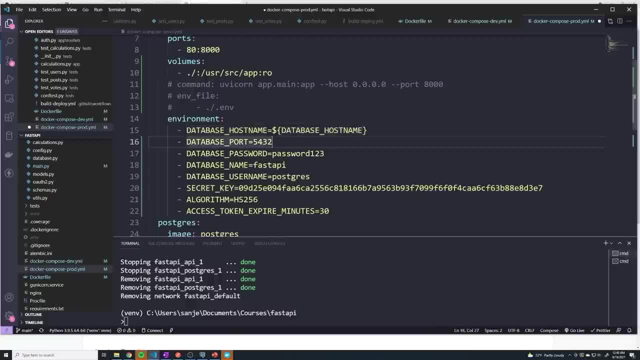 So it's going to look on the you know Linux machine that it's running on for a environment variable called database hostname. So I figured we would just have the match just to show you what that would look like, And then we're going to do the same for all of these. 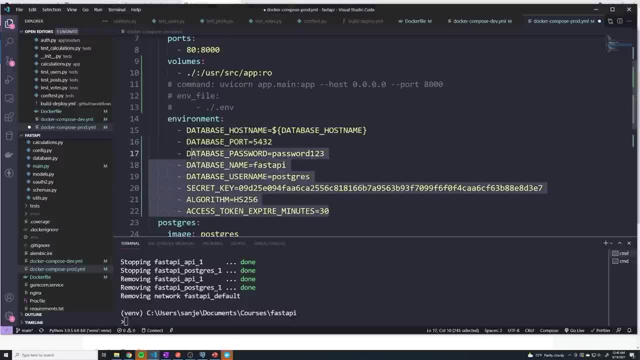 And I'm just going to copy and paste this once again. So it's going to look like this. So it's just grabbing the data- the environment variable- from the local machine. Keep in mind, they don't technically need to match, But it just makes it easier for troubleshooting purposes. 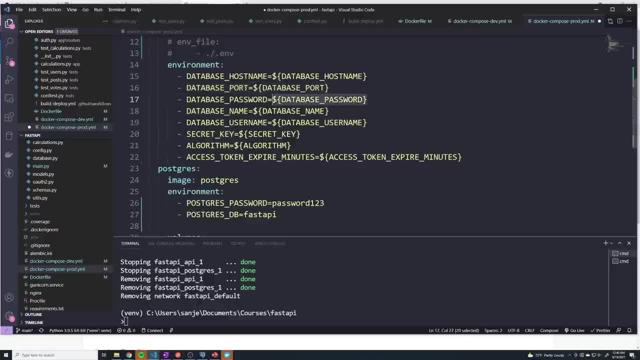 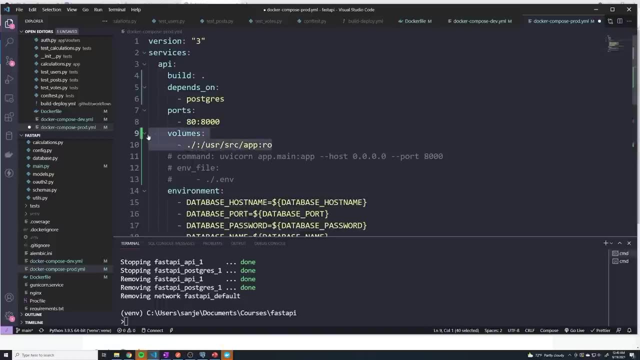 And then for the Postgres database, right, we will want the password to be the same environment variable And then we would on the database name that we're not hard coding that one as well And we don't want the bind mount, So we will remove that. 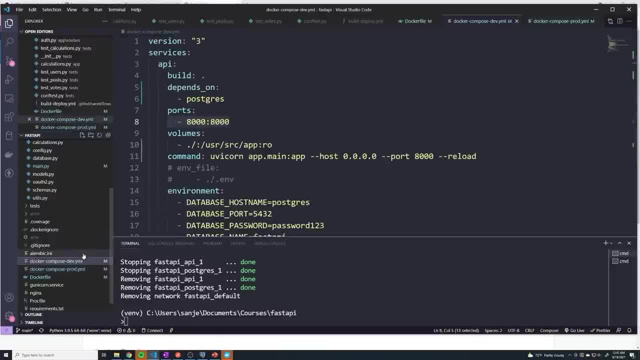 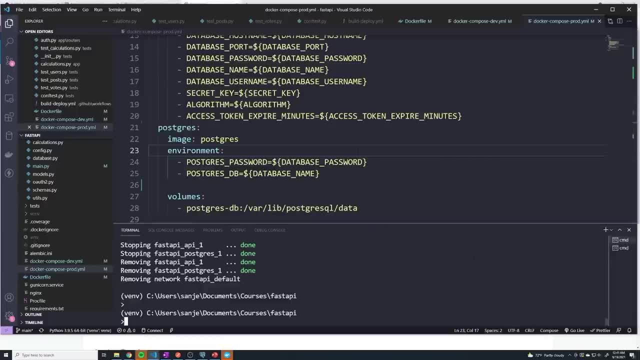 And that's about it. So that's all you have to do. So this just gives us both a development environment and a production environment. We'll save all of that Now. starting up Docker compose is going to be a little bit different now, because we don't. 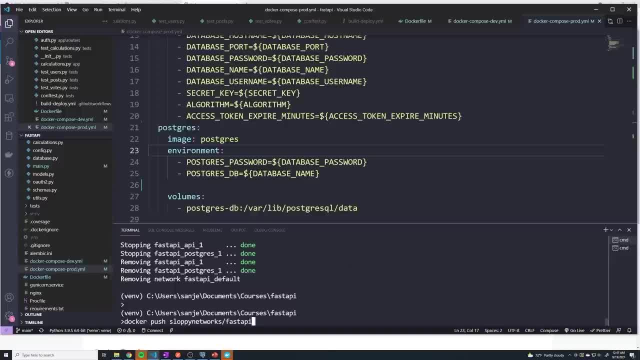 use the default Docker dash compose, dot yaml file name. So if I do a Docker compose, if I can find the up Docker dash compose up, you're gonna see that That just throws an error right Because it says it can't find a Docker compose dot yaml or dot yaml with an A or compose. 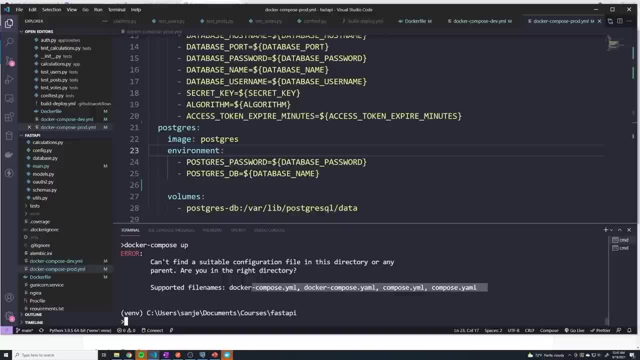 that yaml or compose that yaml with an A, So it looks for only these file names. So when we have a custom file name we have to do Docker dash, compose, And then we pass in the dash F flag for the file name And so we provide the path to the file. 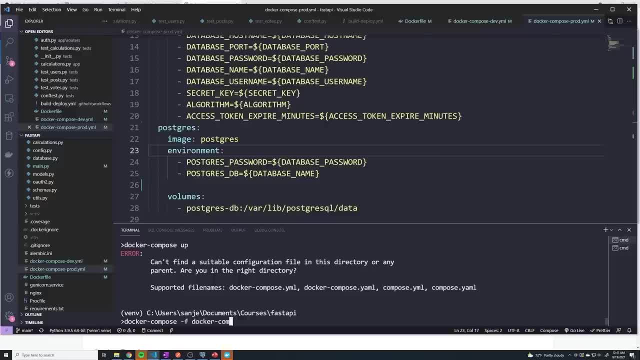 So it's just in the current directory. So I could just do Docker dash, compose, dash dev dot yaml, And then we just do an up and then dash D, And then we can start, Start it back up, And if you want to bring up a production environment, then you would do dash dash prod. 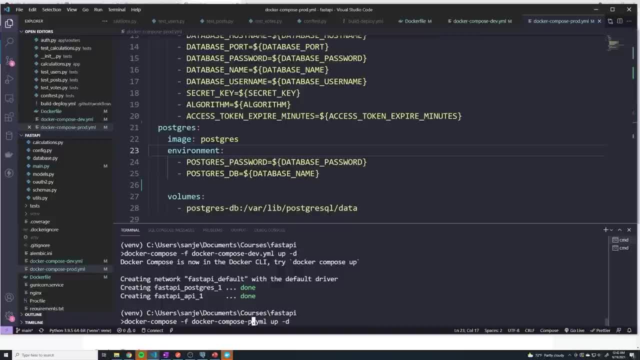 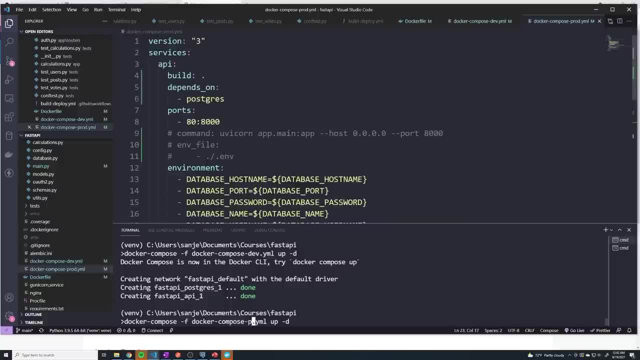 That's the only difference, So you don't really have to do anything else other than running the different specific Docker compose file. And the last thing that I want to change is actually in your production environment. you don't actually ever want to build the image in a production environment. 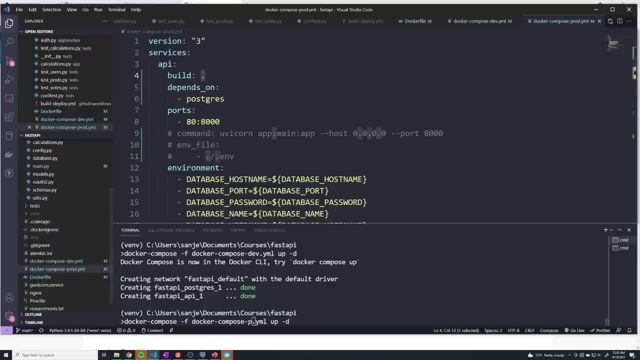 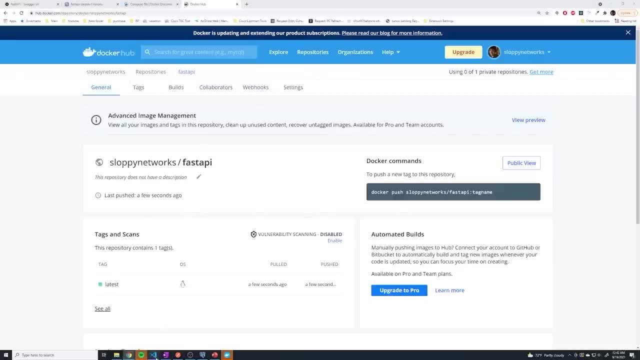 Instead, what's recommended is that when you're done developing, you push the brand new image to Docker hub right And then in the production environment, we just pull this image from Docker hub. So how do we pull this image from Docker hub? 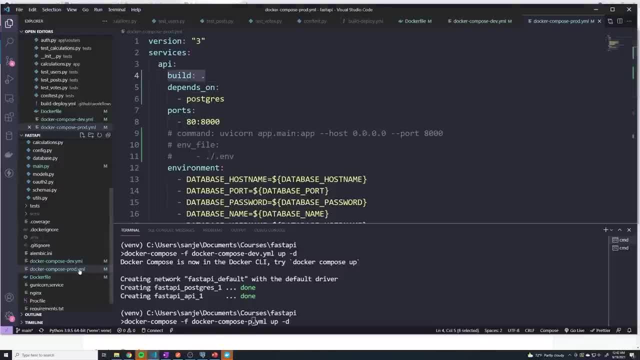 Easy, we change, we remove this build option. remember this is going to be in the prod file And we set this to be a image And here we just set this to the name of the repository. So we just do. you know your username. slash fast API. dash, not dash app, just fast API. 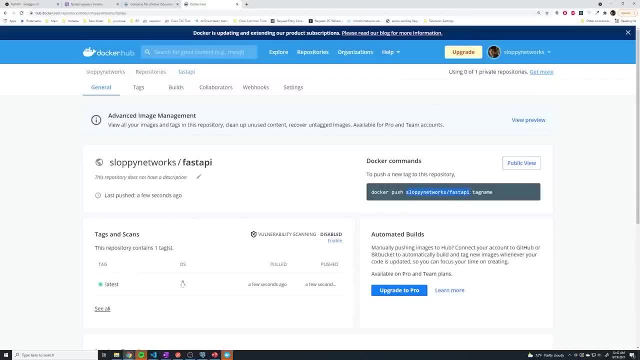 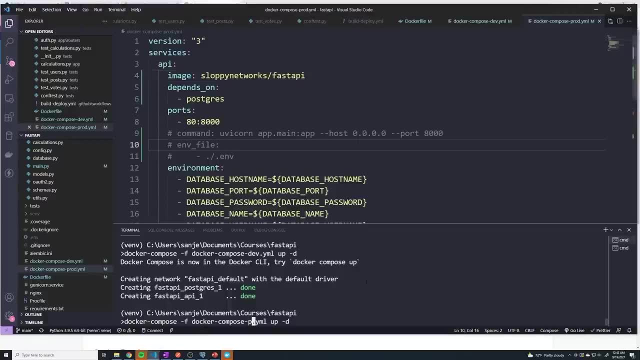 So whatever is essentially right here And then, if you want a specific image with a specific tag, then you would add the tag as well, And so that's all we have to do. feel free to stop your containers now, if you want. And even when you do a data down, you want to make sure you do a dash F, So it knows. 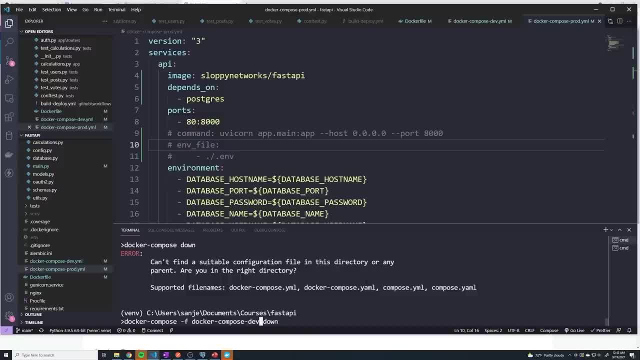 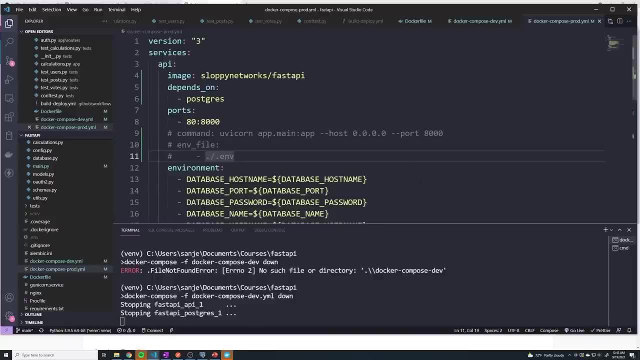 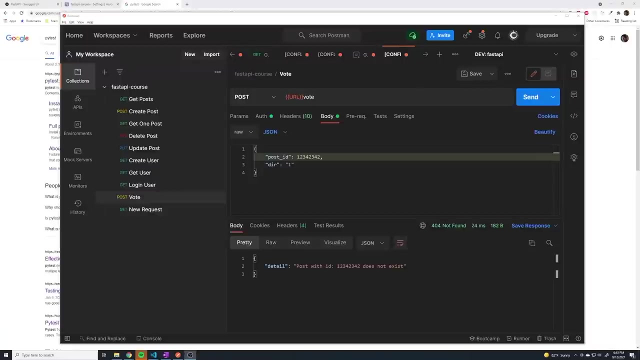 which file to actually look for, And I misspelled that. And that's going to conclude the Docker section of this course, And so I think this is going to give you a solid foundation on how to dockerize your fast API Now. currently, whenever we make changes to our code, whether it's implementing a new 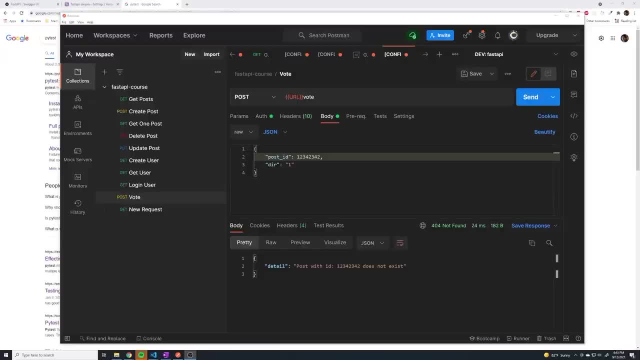 feature, or modifying the behavior of a previous feature, or even fixing some bugs that we happen to catch. we have no idea if the changes we make break other functionality in our code, And so normally, anytime we make any changes, we then have to, you know, go into postman. 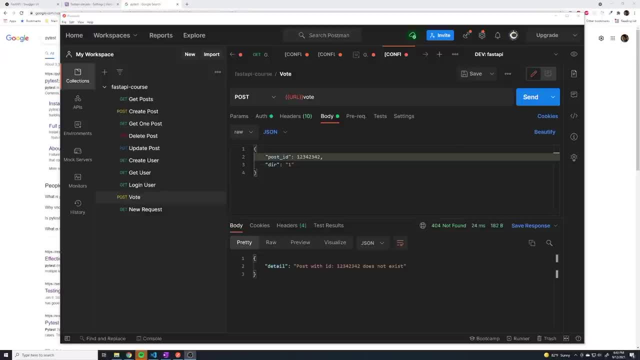 and essentially manually test out every single scenario to ensure that things are working, And this isn't a very scalable solution. it's going to result in a lot of wasted hours. for every single time you have make any changes to your code, you're going to have to test. 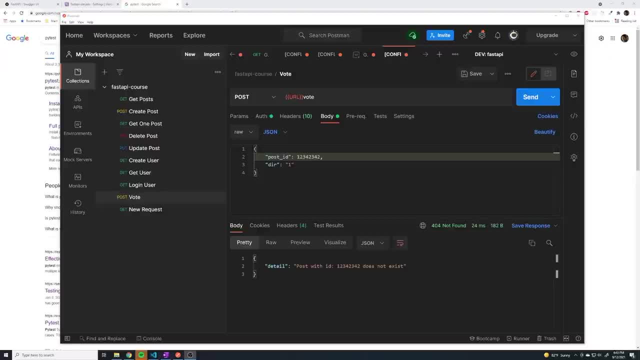 everything because you don't know what, what code you've broken by making those changes, And so this is where you know an automated testing library comes into play where we can define a whole bunch of tests to test a majority of the functionality of our code. 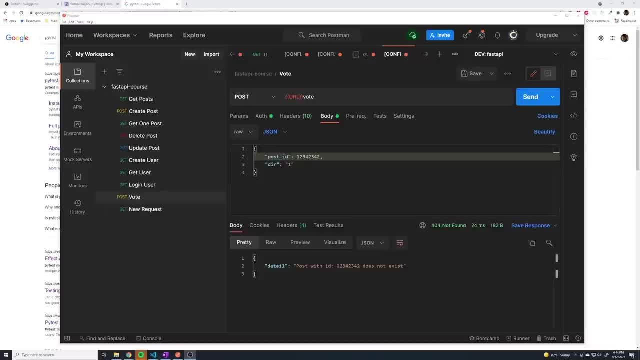 And so that way, anytime we make changes to our code, we can really test the functionality of our code, We can run our tests to see if we've broken anything And keep in mind. you know, obviously we can't test for everything. 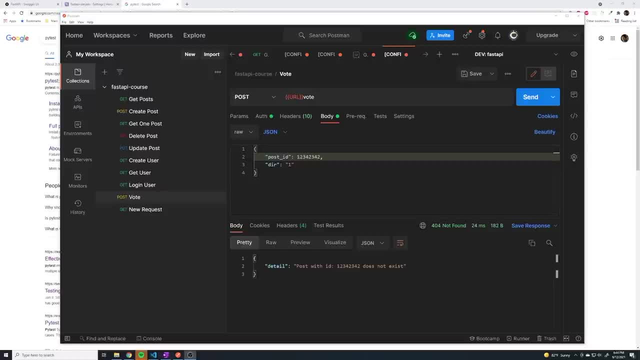 But we can at least test for enough things that we can catch some of the more obvious bugs, And so this section of the course is going to be dedicated to getting started with testing and really understanding the concepts of testing and seeing how we can get started with a library. 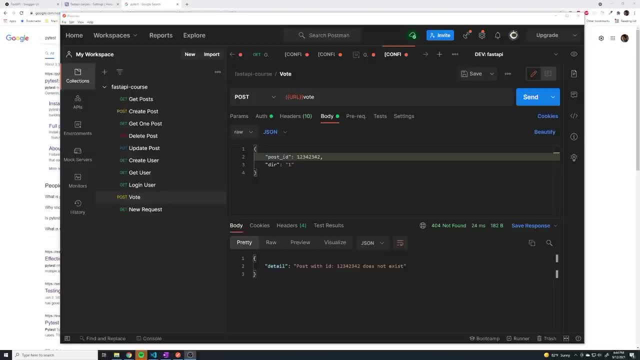 like pi test, But I do want to provide one little disclaimer before moving forward. I wasn't originally going to post a section on testing for this course, And the reason for that is that I don't have much experience with testing. It's not something I do a lot of, or in or at all. really. 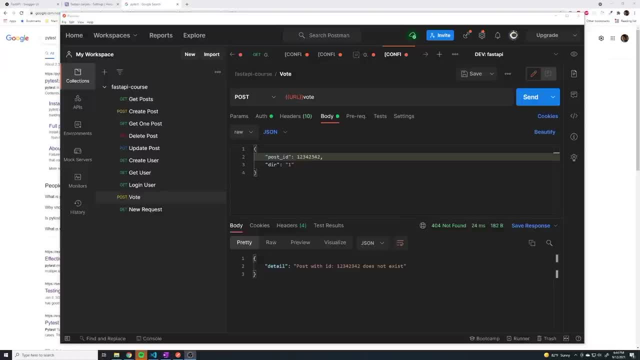 And so I want to make sure that you guys understand where I'm coming from when it comes to testing, And that is that. you know, since I am not super proficient at testing, you know, I don't really feel too qualified to actually teach it. 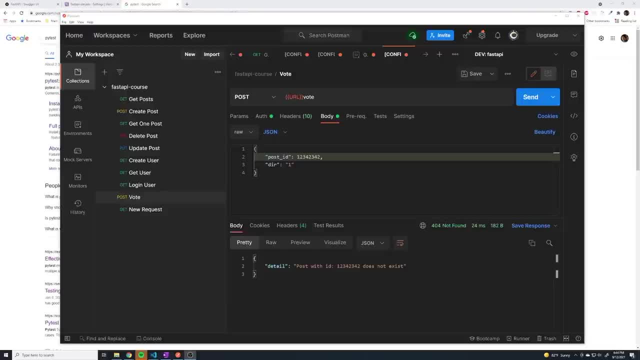 And so what I want you guys to do to take it, what I want you guys to take out of this section of the course is just to how to get started with testing. How do you set things up And what's the main ideas behind a test? 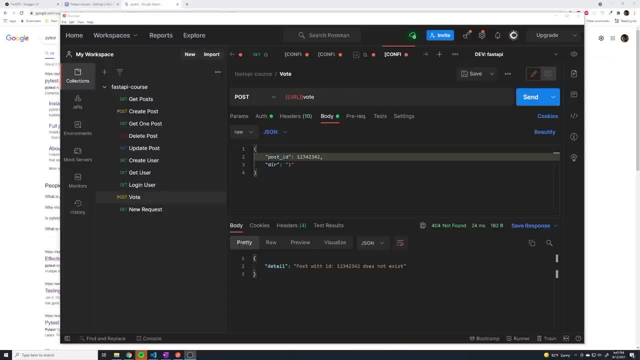 I may not necessarily be teaching the best, most efficient way to test, I may not be test using the most efficient way of testing And there may be scenarios where I may not even be following best practices. But I want to show you guys how we can at least get some integration tests set up. 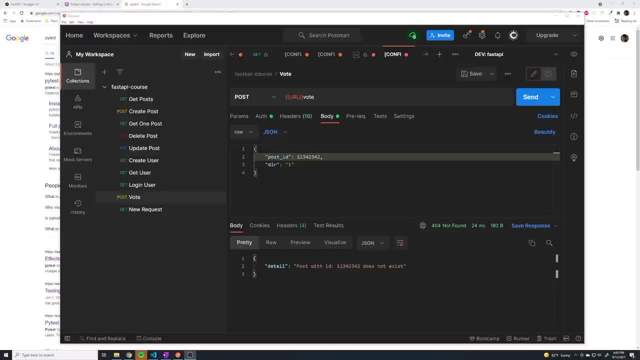 And then, at that point, what you guys can do is you can just forget everything else that I've taught you when it comes to testing. Once you at least have the groundwork, then you guys can, you know, do your own research, figure out how you ultimately want to implement testing with any of your projects, and then 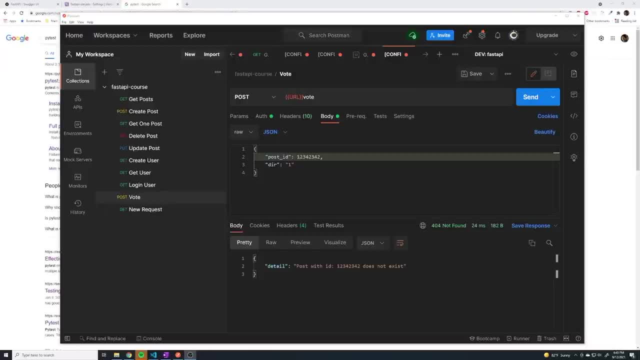 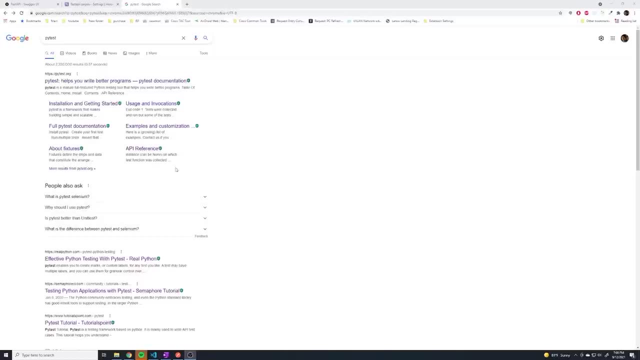 go ahead and just run with that, Okay. So with that in mind, in the next video we'll get started with getting PyTest installed and writing our first test For testing the library that we're going to be using is PyTest. 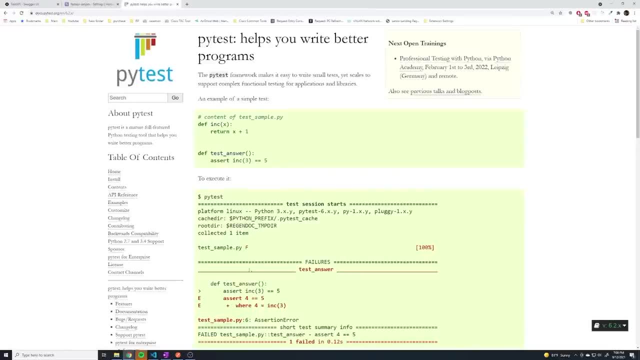 So if you do a quick Google search, you can just search for PyTest And the first result is going to take you to the documentation page for the PyTest library, And so I recommend you guys take a quick look at this just to see how it gets set up. 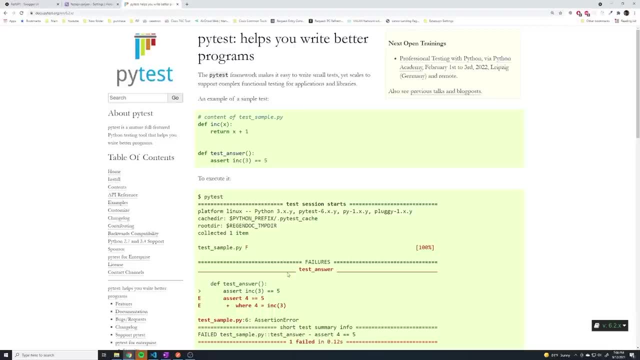 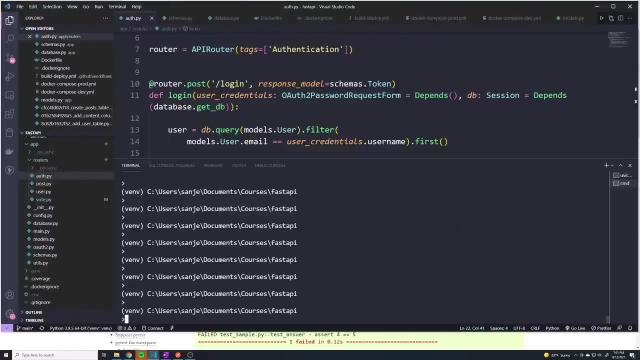 And if you want to do a little bit of reading before we actually get started writing our first test, definitely go ahead and do that. But once we've got that Opened up, what we can do is we can install PyTest. So we can just do pip, install PyTest just like we would with any other package. 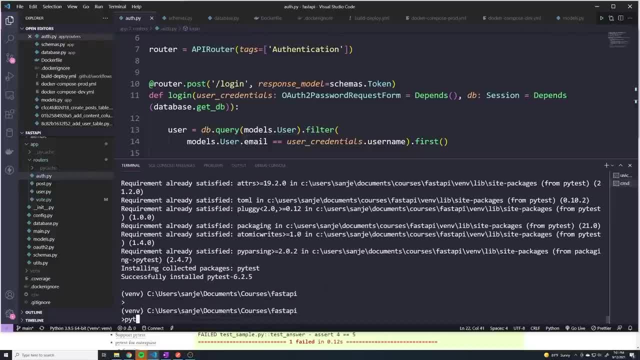 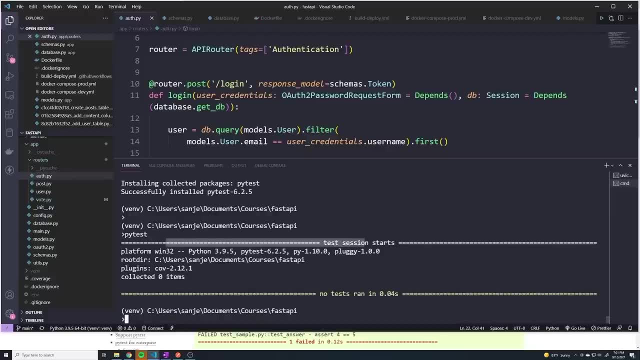 Then, once that's done, we have access to the PyTest command. So just go ahead and run PyTest and see what happens. So print out a few things. you notice that we can see that the test session starts. So this is when we start testing. I print out some information about the platform that 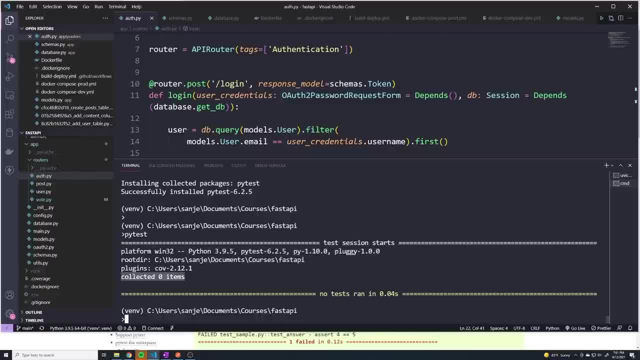 we're running on And that's okay. we can ignore all of that And you'll notice that it says collected zero items. We'll talk about this in a bit. But the more important thing to look at is it says no testing. 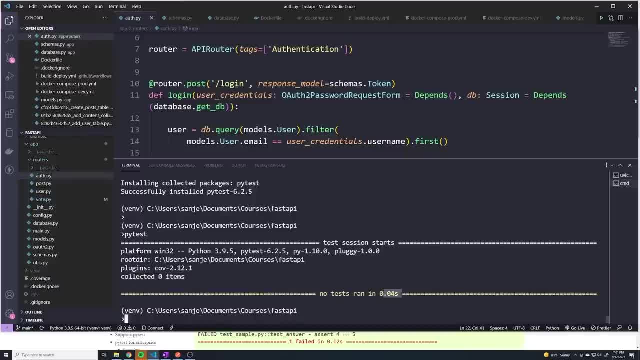 No tests ran in point zero four seconds, And this is expected. you know, we haven't created any tests, So obviously it's not going to be able to run any tests. But to run our testing, all we have to do is just run this command. 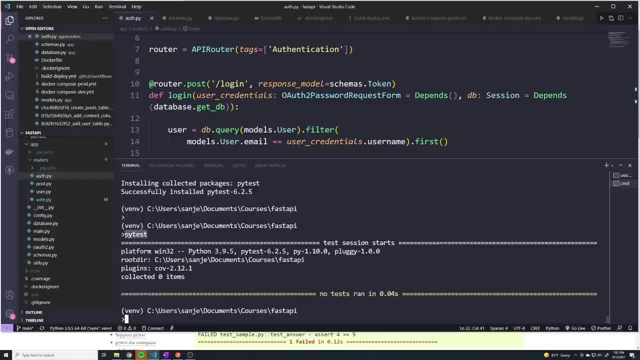 And then you'll see that PyTest will go through all of your tests, run it to verify. you know that they all pass And if there's any errors or anything like that, it's going to report that. So it really is as simple as that. 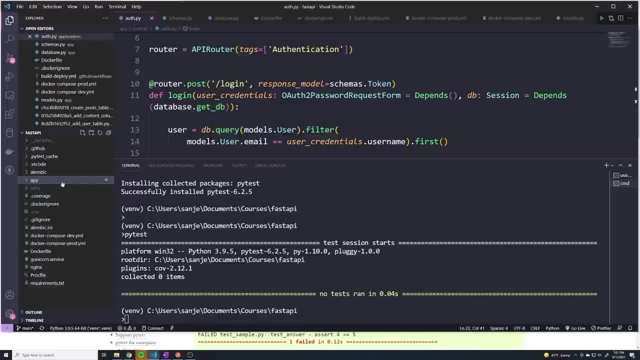 But let's go ahead and create our test, And I want to store our, all of our tests inside a directory called tests. So inside the root directory of your project, just create a new folder. we'll call it tests And technically you can put this folder anywhere. 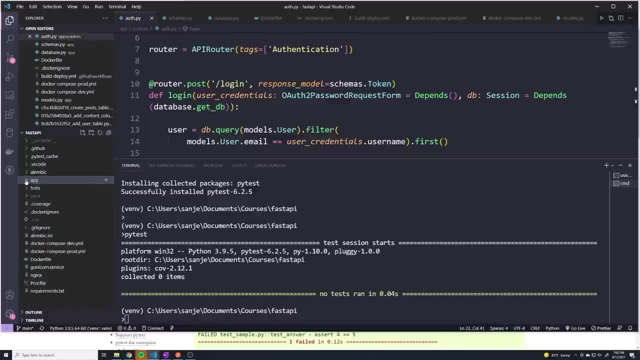 If you wanted to put this test directory within your app directory, you absolutely could. It's a matter of personal preference. I'm just going to keep it outside of the app directory for now, And within here I'm going to actually create a file. 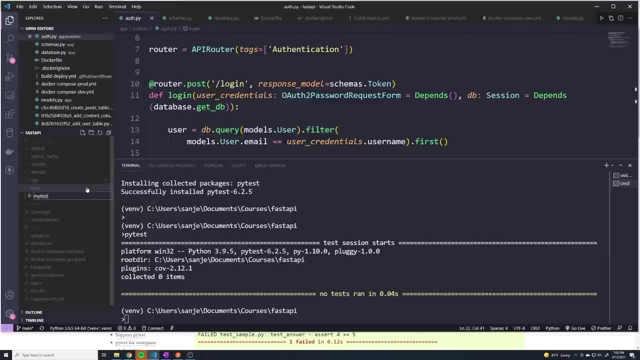 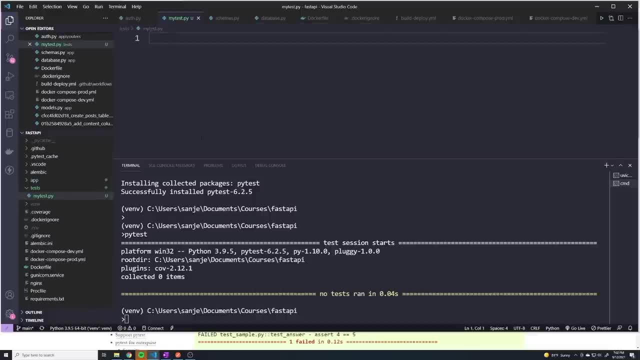 And this is going to store our first test. I'm just gonna call this my testpy for now. Alright, And we obviously need to test a part of our code, whether that's a route or a path, operation or a function or a class. we need to test something. 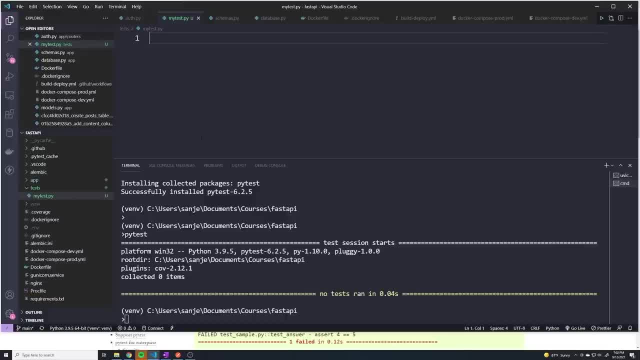 And right now our code is a little advanced, And when I say advanced, I don't mean advanced, because anything we've done is super advanced so far. It's advanced from the perspective of testing, where we're coming in from a background of no knowledge of testing. 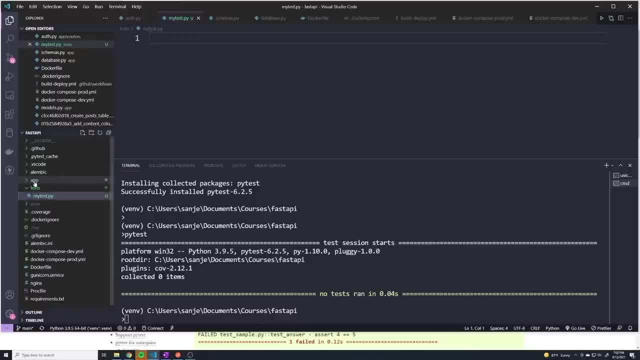 So we want to start out with testing the simplest functions. So I'm going to actually create a brand new module and essentially create the simplest module or function that I can possibly think of. So I'm going to create a new file. call it whatever you want. 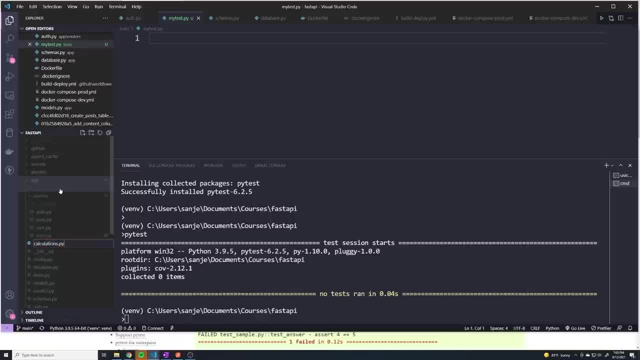 I'm going to call this calculations, because it's essentially going to be a bunch of functions that we use to perform certain calculations, And I'm going to define the world's simplest function, which is called add, And I think you can guess what this function is going to do: it's going to take two numbers. 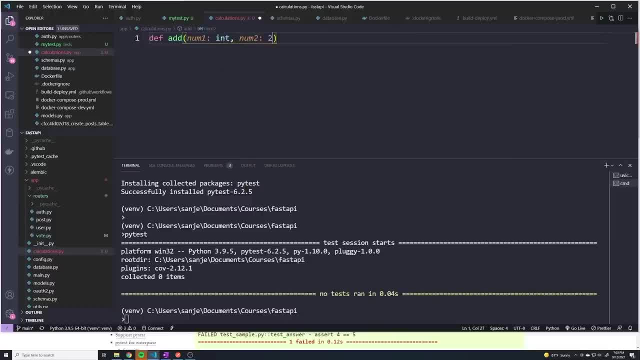 which is going to be type int And it's just going to return the sum of them. So we just say return num one plus num two. And the reason, once again, is because this is going to be a very simple when it comes to testing. 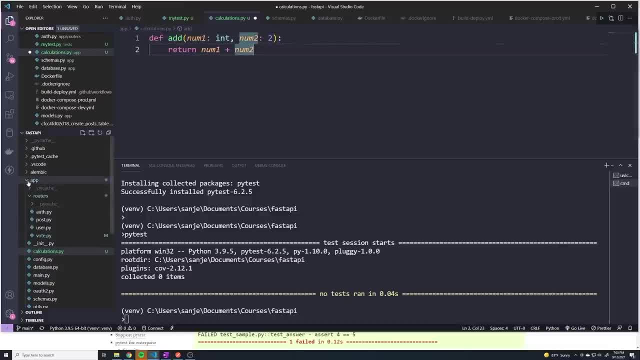 So you guys can at least have an understanding of how to actually perform these tests. So we've got this module defined inside our app directory And then, in our tests folder, we've got our my testpy And we're going to define our first test. 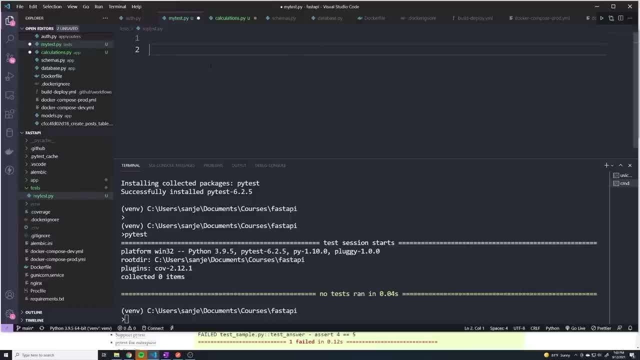 So what is a test? Well, it's really just a function. It's either a function or a method within a class. we're going to start off with just doing functions, because it's just a lot easier, And we're going to call this function test, underscore add. 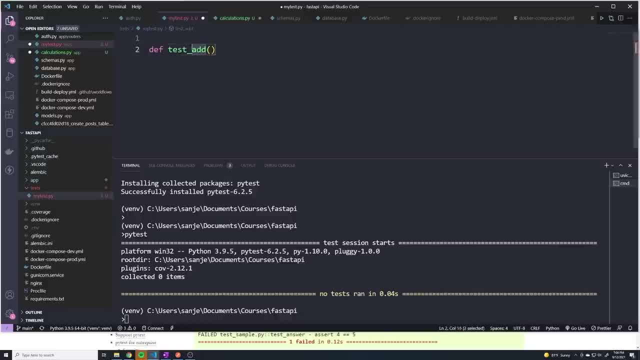 Why did I give it that name? Well, it's testing the add function, So I think that makes sense. And technically, the name, the naming, does matter, But we'll come back to that in a bit. Now, how does this function actually work from a testing perspective? 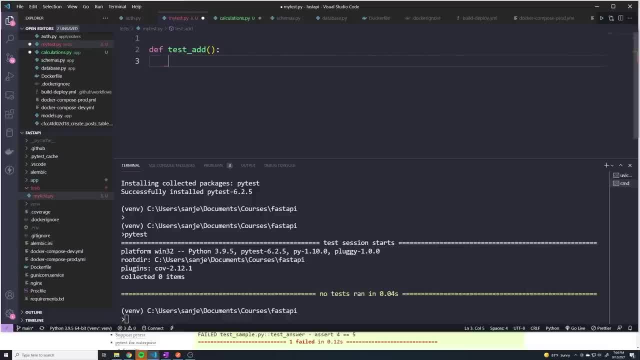 Well, it's very simple. You know, pi test will run through all of our tests And when it runs through this specific test, what it's going to do is: if it runs through it and there's no errors get thrown, That means the test has passed. 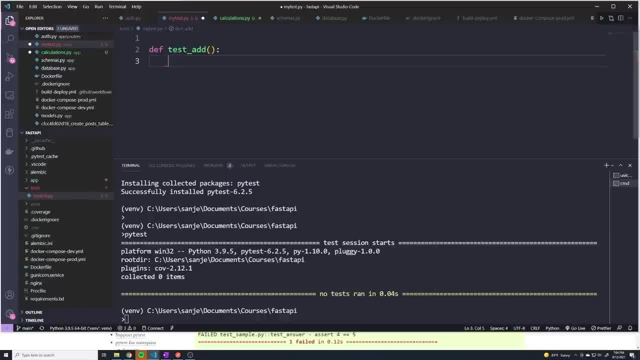 It's succeeded, that means our code is good. If our function throws an error of any kind, it's going to consider our function or our test as failing. then the test has failed. So how exactly does that work? It's a simple. it's simple: we use something called assert. 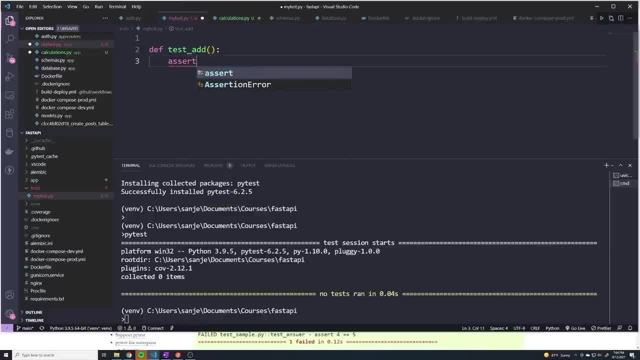 And if you aren't familiar with what the assert command does in Python: anytime you assert a true value, nothing's going to happen. the code just runs. However, if you assert a false value, Yes, it's going to throw an error. 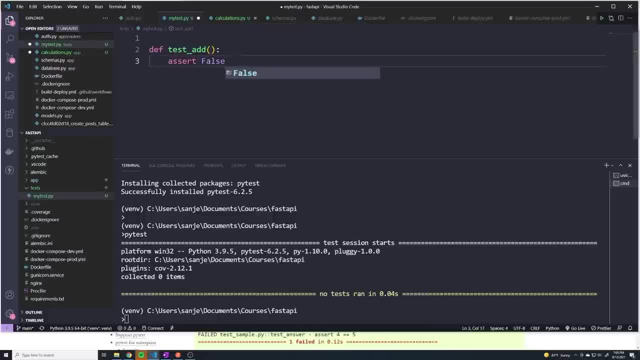 So it's. it's no different than raising an error or throwing an error In Python. it's just a simple way of doing that for testing purposes. If we return something that's true, then the assert won't do anything. If we return something that's false, then it will raise a Python error. 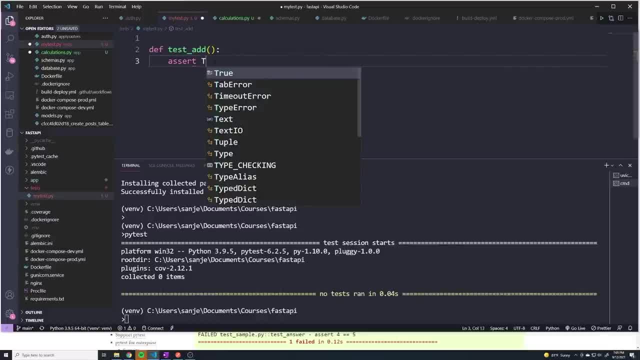 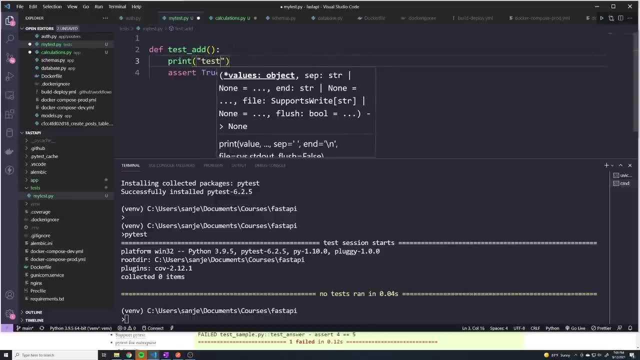 And I'm going to show you exactly how that works. So if I just say assert true, and before this I'm just going to do a print testing add function And then down here I'm going to just call the test underscore add function, right here. 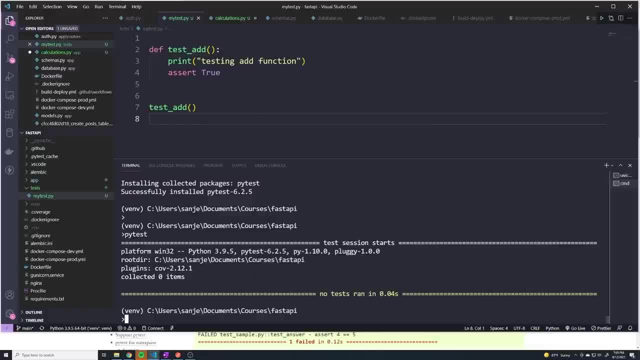 And I'm going to just run this as a normal Python module. So we're not going to even treat it as an actual test or anything like that. We're not even going to use pi test, So I'm just going to call Python. 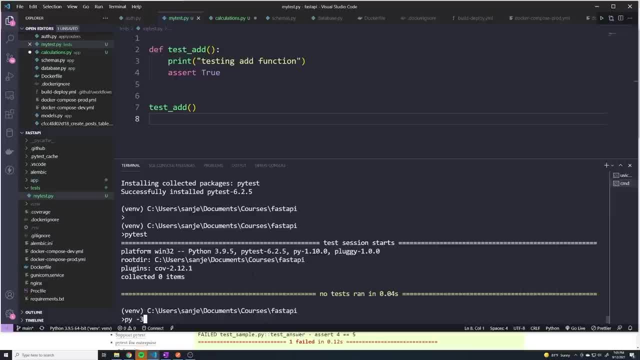 And keep in mind that the command is Python on on Mac, but it's pi dash three on Windows. And then we're going to go into the test directory. I want to call my my test py and I'm going to show you what happens. 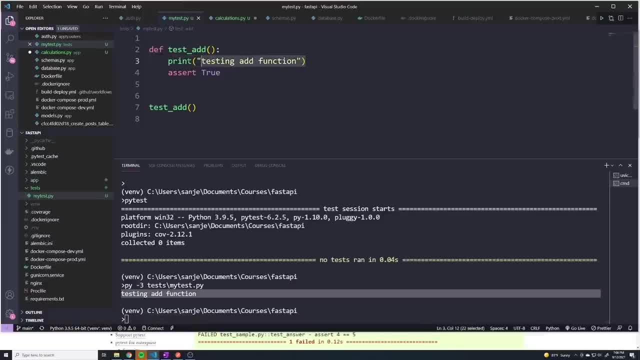 All right, we can see it says testing add function, which is from this print statement, And then you can see the assert did nothing, So it just ran and everything's fine. And that's expected because, like I said, assert only does something when we return a false. 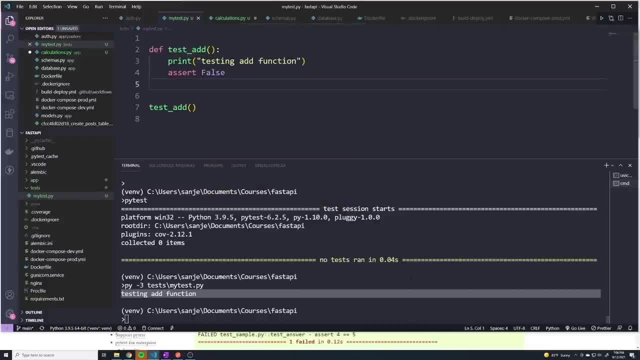 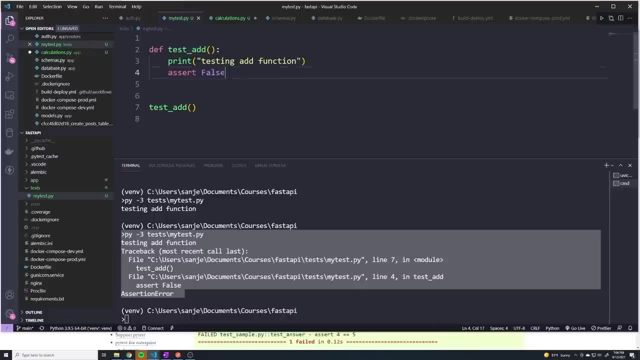 value. So if I say false now and I run this code, take a look at what happens. Hey look, Python throws an error. So assert is simple as that. true means nothing's going to happen, false means it's going to throw an error. 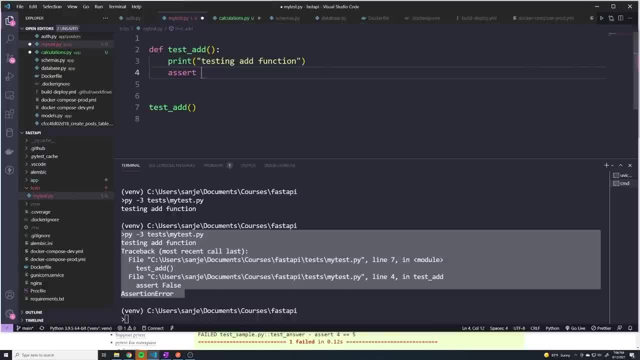 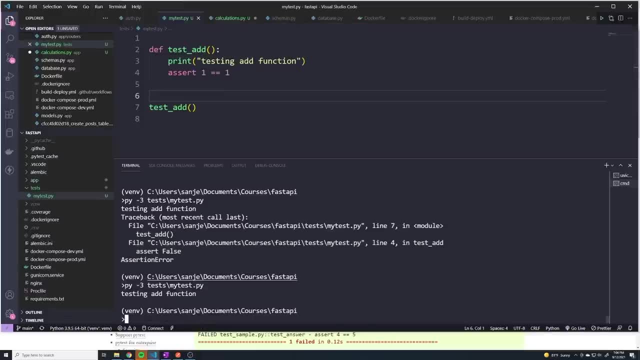 And we don't have to just say true or false. we can actually pass on a condition. So if I say one equals equals one, that's going to return true, right, So technically an assertive true won't do anything. However, if I say one equals equals two, that's going to be a false statement. 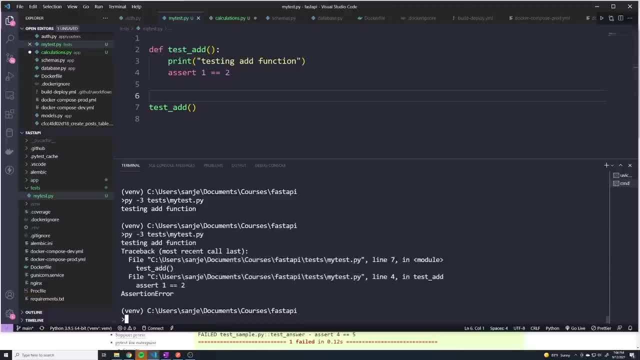 And if I run that, we can see that it asserts and it throws an error. So that's how we make use of assert within our testing functions. So I'm going to remove this And we're actually going to test out our code now. 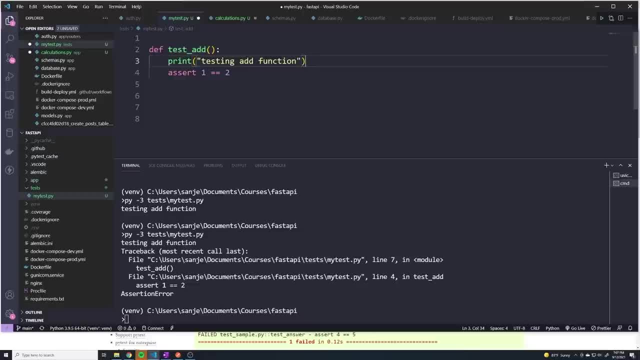 So there's a little bit of a delay. So to test out our add function, the first thing that we have to do is we actually have to import it into this file. So we're going to import it, So we'll say from, and we have to go into the app directory and the calculations model. 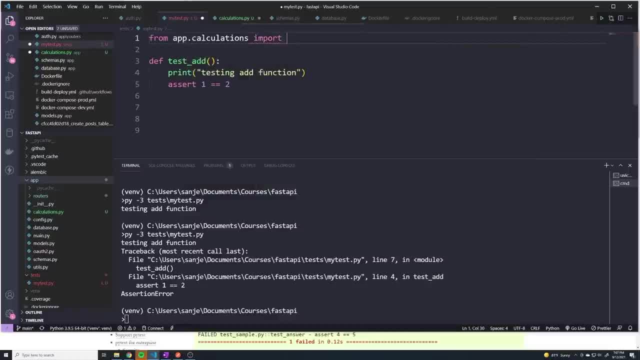 module. So we'll say app, dot, calculations, import, add. And now what we're gonna do is we're just going to call the add function, like we normally do, And we need to give it some test data. So I want you to think of two numbers that you want to use for testing, add them up and 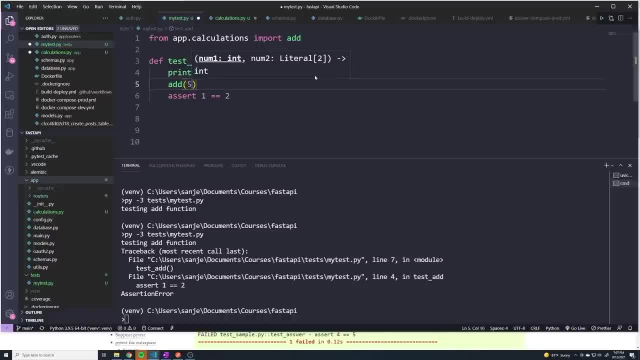 what is the result? Should it be So? I'm going to say I'm going to do five and three, And I know that this function, if it works properly, should return a value of eight, because five plus three equals eight, And so I can just take the sum, store that in a variable called sum. 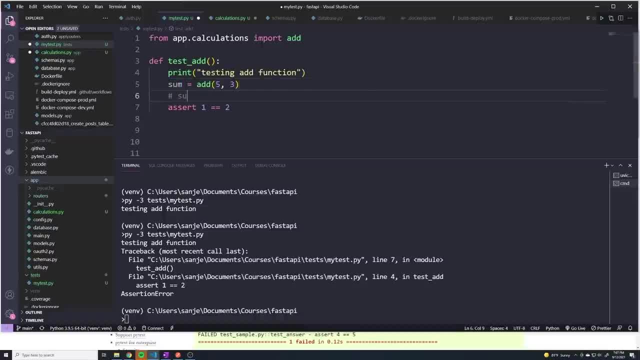 And what we can do is, since I know some should ultimately be equal, equal to eight. I can assert that and that, should there should be no either, So I can say: some equals equals eight. So that means, if, If our code runs fine, some should ultimately equal eight. 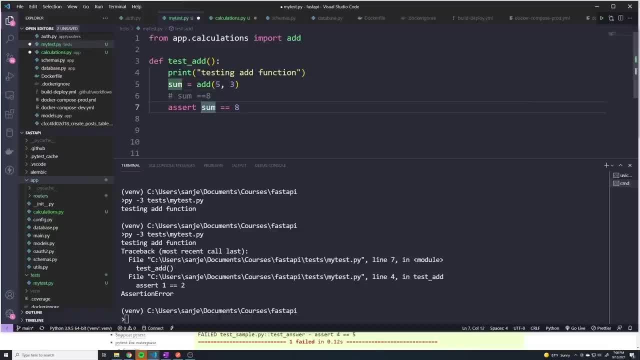 And if we assert eight equals eight, that means it's going to return true and nothing should happen, or pi tests should consider it as passing. However, if I mess up my code and, for some reason, the add function returns a value of 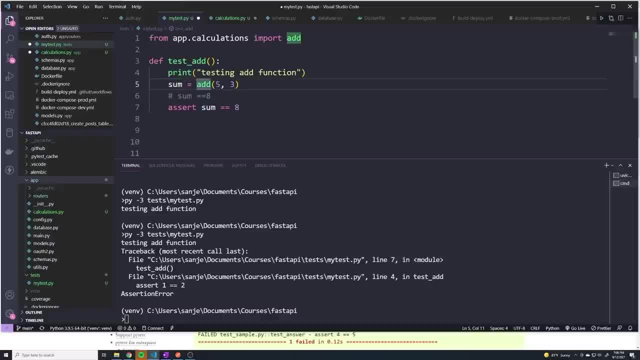 20, then when we do assert 20 equals eight, well, that's going to be false And it's going to throw an error and it's going to consider that as a failing test, because an error means a failed test. So that is the main idea behind a simple 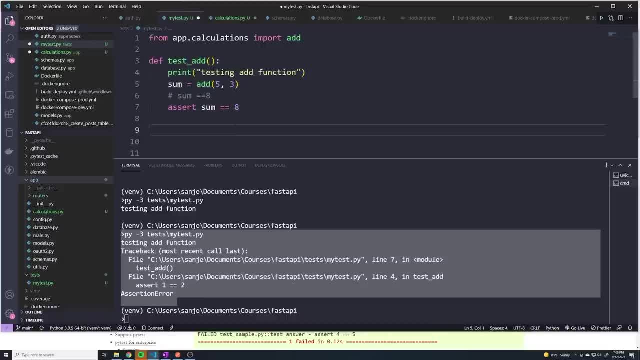 Automated test within pi test right. You just provide, you run the code with some test data And you know what the result should be, because you created this test data And you just make sure that the result of the code matches with your expected result. 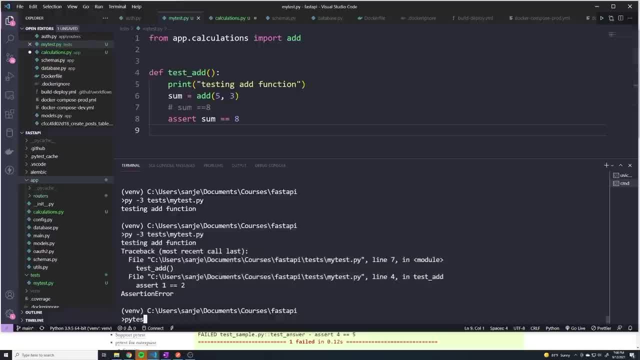 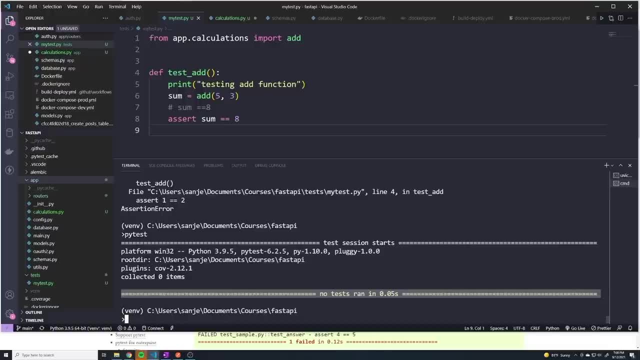 So let's actually run our test now. So I'm going to do pi test and let's see what happens. Right, And you see, the same exact thing we saw before. Once again, it says it collected zero items, no tests ran. 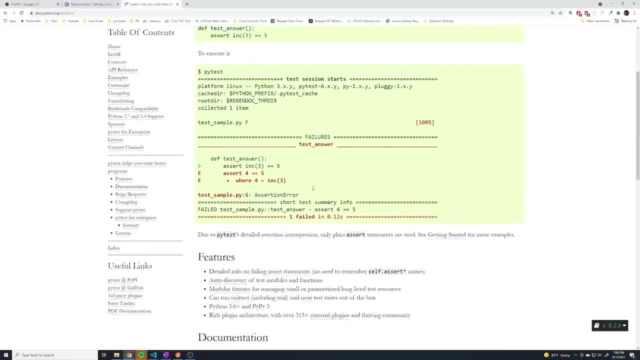 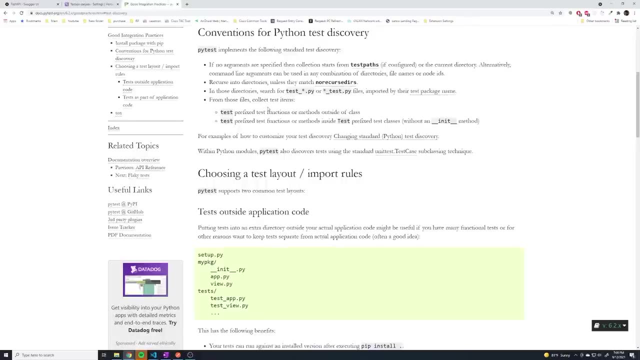 And so why exactly is this happening? Well, if we go to our documentation and you scroll down to this feature section, you go to the auto discovery section, And so this auto discovery section is going to explain how pi tests finds all of the tests. 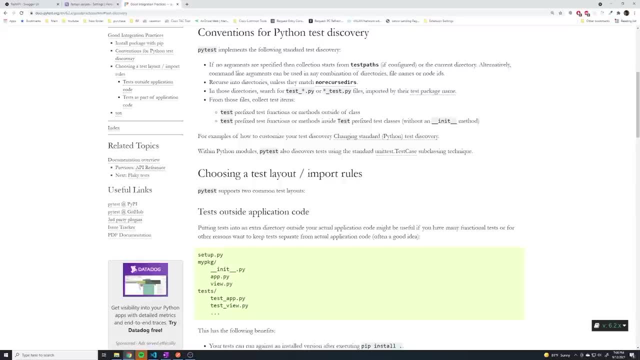 in your code because it does have a auto discovery functionality where it can actually go through all of your code, all of the directories and packages and recursively look through them and find the tests. but it looks for specific keywords And you can see in these directories it looks for any files. 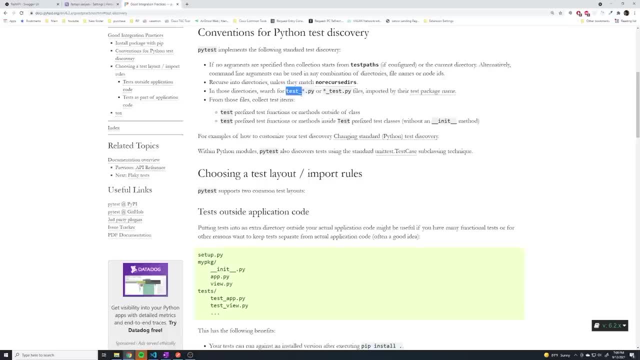 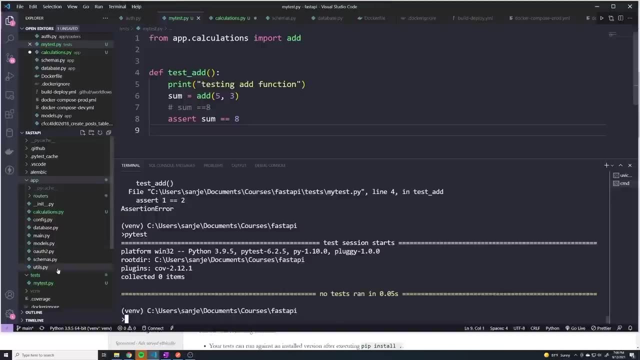 Let's start with test. So you have to do test underscore and then some name or some name underscore testpy. And if we go to our code right, we named this my test. this does not match what it's going to look for. 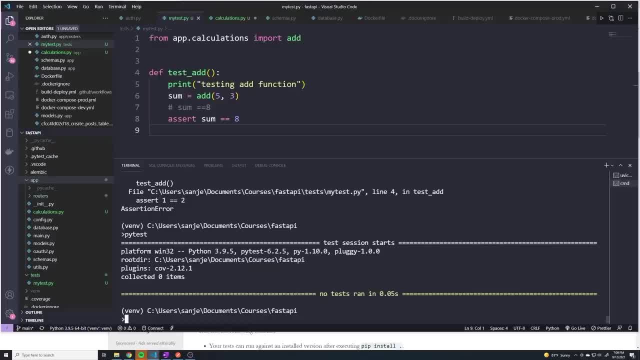 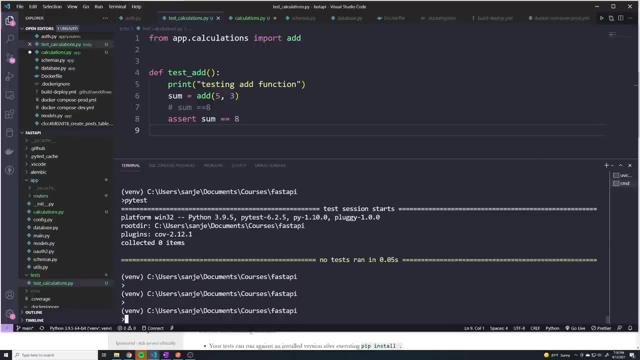 And that's why it doesn't actually find any tests from that. So let's change this, I'm going to call this, let me rename this, and I'm going to call this: how about test underscore calculations? Alright, and so now, if I run this, you can see that it throws an error. 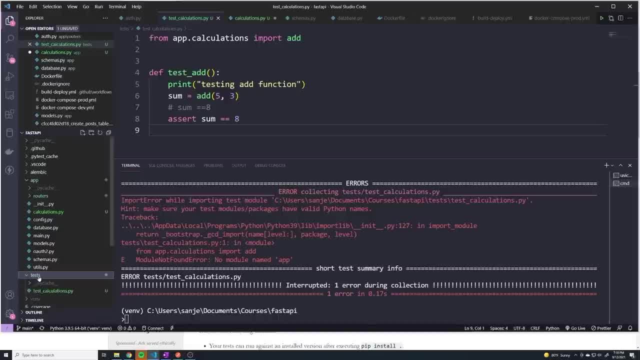 But I realized that, you know, within my tests package, I do need to have the usual underscore in it, underscore, underscore, dot p y to actually make it a package. So I'm going to do the same thing. I'll do underscore, underscore in it, underscore, underscore dot p y. because of that it wasn't. 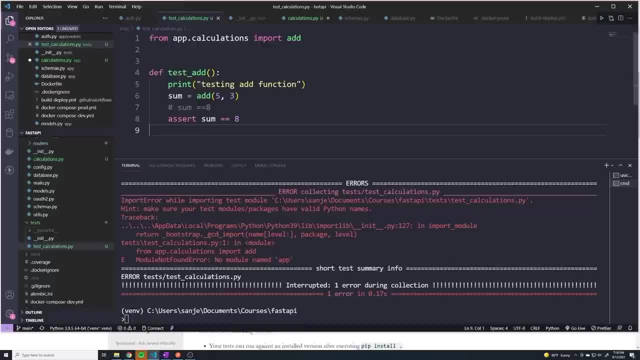 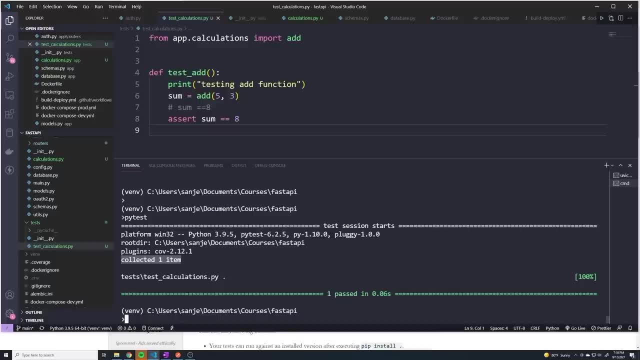 able to actually import the file properly. So let's, let's save that And let's try this, Let's try this again. So now, if I run this, you could see that, hey look, we collected one item. So I think it's safe to say that this collected one item and probably means we have one test. 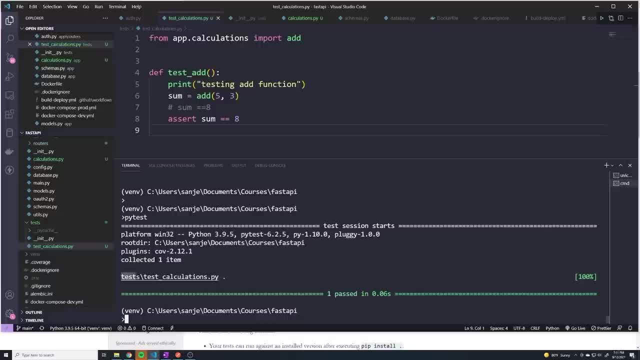 So the number of tests equals items. And then we can see that inside the test package we have a module called test underscore calculations, dot, p, y, And then there's a little dot. So the dot reference represents one individual test And a green dot means good. 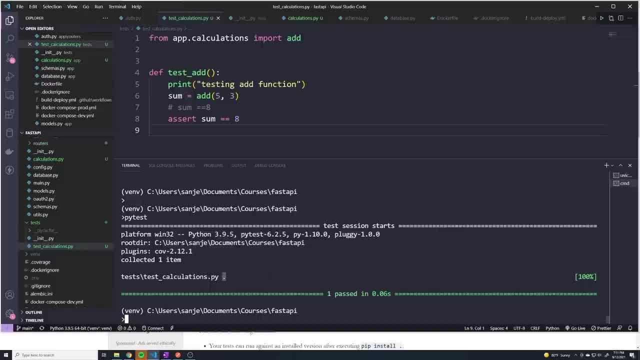 A red dot means it failed, right, Green is passed, It failed. And so if you have two tests, then you would see two dots, And then if the second test pass, it would be green, If it failed, it would be red. 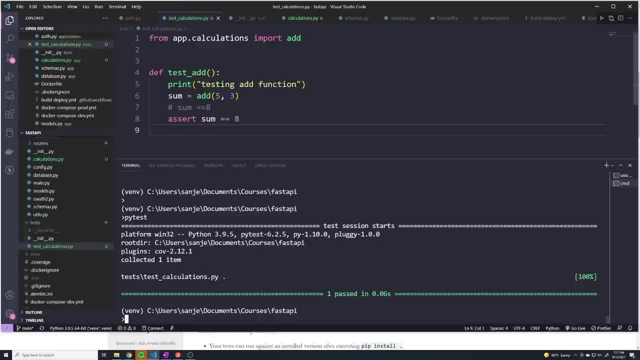 Simple as that. And so now we have successfully ran our first test, And just to make our code a little bit simpler, right, I could just, instead of having the sum variable, I can just cut this out- just paste it into here, just to make it a little. 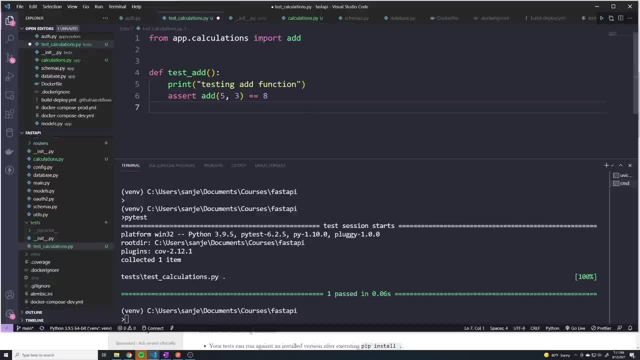 bit cleaner, And then we can remove all of this. And just to make sure I didn't break anything, let's run our test again And we can see that once again, it worked Just fine. Now, when it comes to the auto discovery of files, a few things to note. you don't necessarily 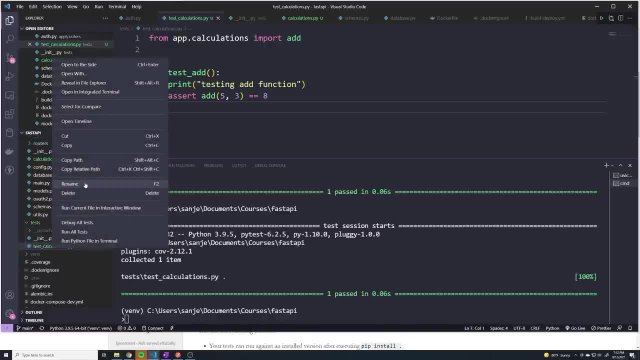 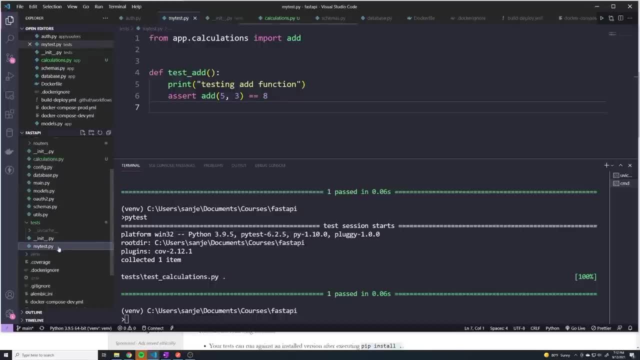 have to follow this convention of test underscore calculations. If I actually rename this and I call this, you know my underscore test, what did I call this? my test dot p y. right now, if I obviously run this, it's not going to find any tests. 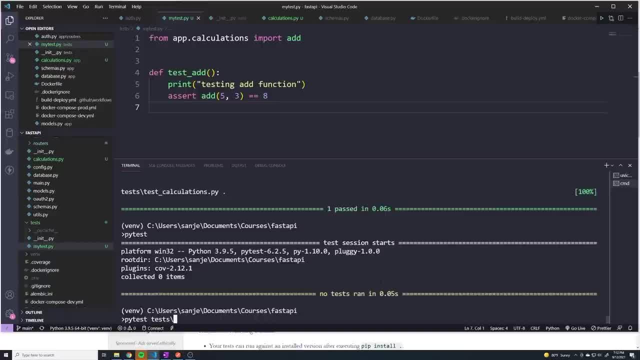 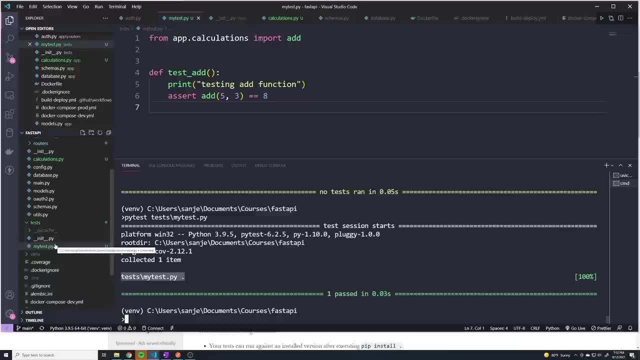 but I can pass in the specific path or the specific module that I want to test. So if I do my test dot p y, then it is able to find the test. But I like to have pi tests be able to automatically find all my tests so that I don't have to specify. 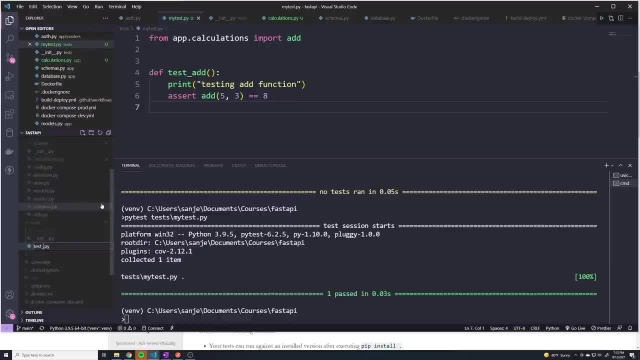 this. So we'll rename this and go back to test underscore calculations, because it ultimately is a module that's going to be testing my calculations module. And another thing to note: the name of the test within the module also matters. If I call this, you know, maybe something like testing underscore add. take a look at. 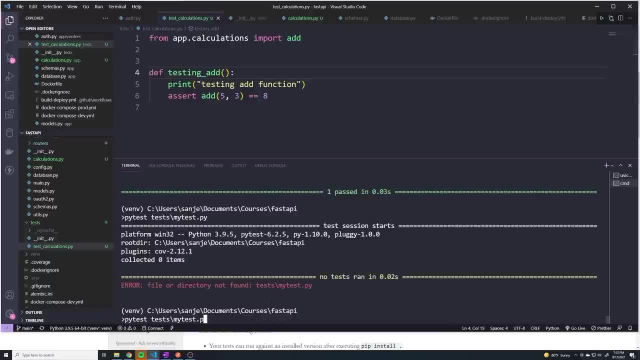 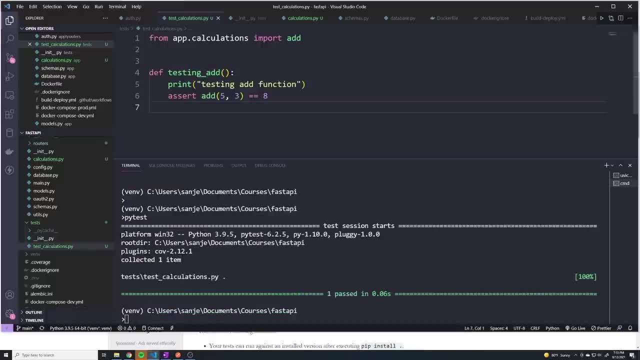 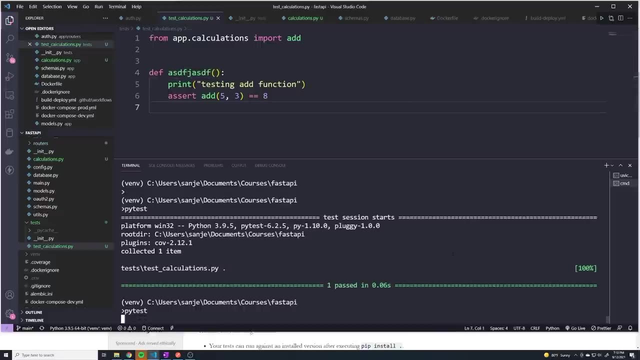 what happens? Whoops, I wanted to auto find it now And I forgot to save it. Now, if I run this, it looks like it still works. But let me change this to just something random, And so now we can see that no tests ran. 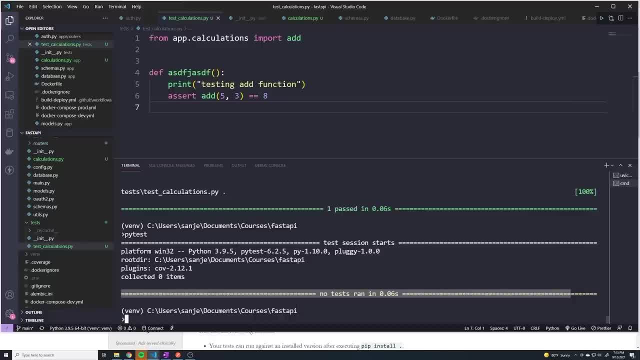 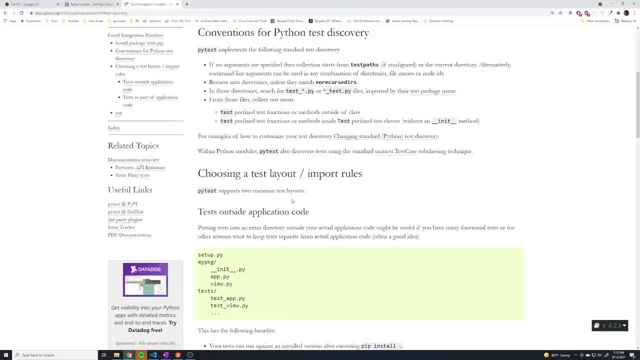 So the naming of the function absolutely matters when it comes to auto discovering tests And you want to stick to the standard of test, underscore something And I think somewhere in this documentation it's going to go over here we go, test from those files, collect test items. 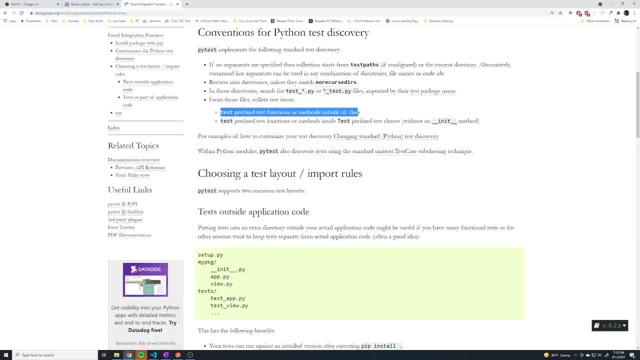 So a test prefix test function or method outside of a class or a test prefix test function or method inside a test prefix test clause. So it's got to start with test. essentially it doesn't necessarily have to be test underscore. That's why testing underscore add worked just fine. 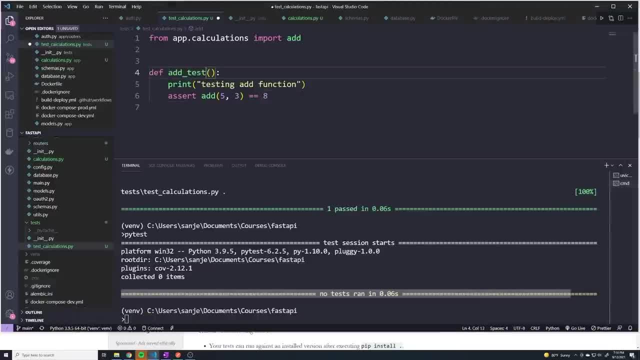 It does have to start with the word test. That's why, if I said add underscore test, I don't think this will work. actually shouldn't based off of their description And it doesn't. So keep in mind that the naming does matter. 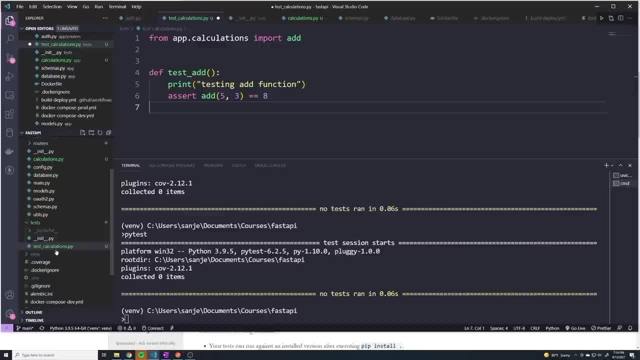 And I recommend you stick to the convention of naming all of your testing modules- test underscore and the name of the module that you want to test, and then your functions- test underscore and then the name of the function that you want to test or the functionality that you want to test. 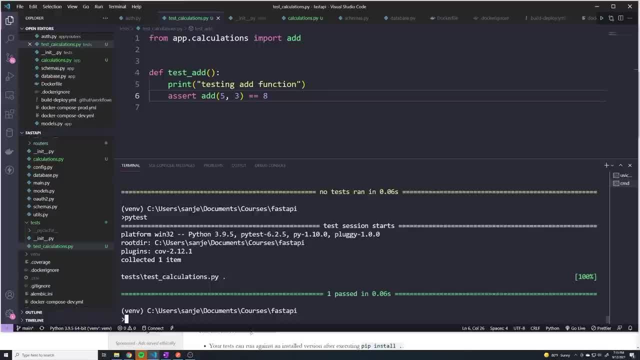 Now a couple of things to note. I'm going to run this test again And you'll see that it doesn't really give us much detail as to what's happening. But we can pass in other flags to get a little bit more detail or to change the functionality. 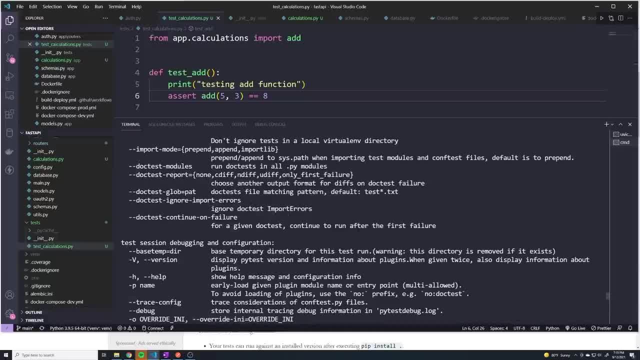 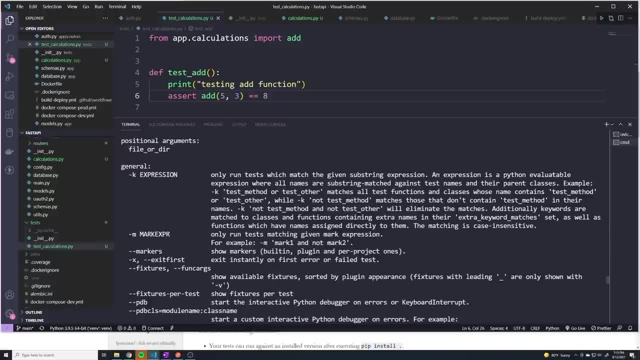 So if I do pi test, dash, dash help- You'll see that there's a lot of options, But I think something that would probably be helpful is like a dash v for verbose, And I think we should have that in here. So let's see if I can find that. 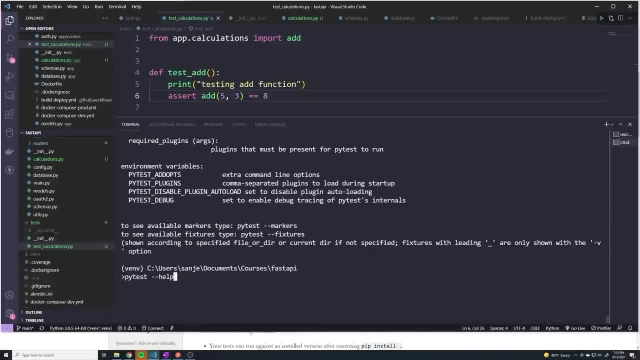 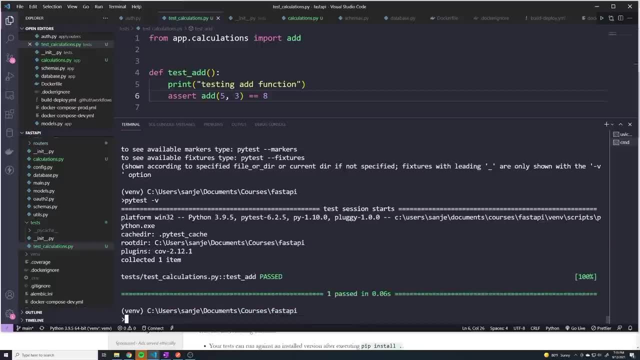 Here we go. Dash v is increased verbosity, So we'll just do pi, test dash v and let's see what happens. And so now, instead of just having a dot, it's actually going to list out the specific test that's running. So I think that's a little bit more helpful. 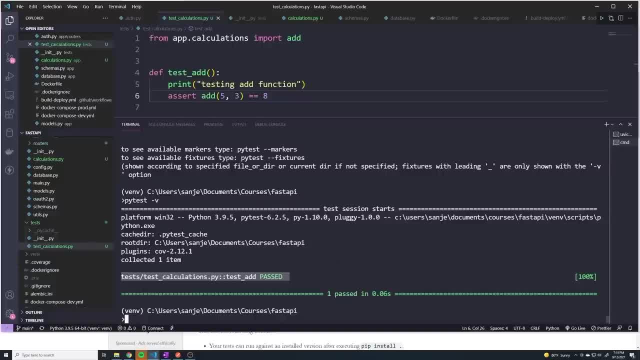 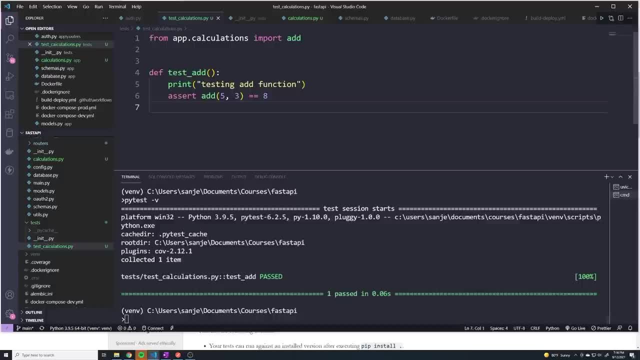 And I usually like to run these tests with a little bit of extra verbosity, just that I know what's happening. However, maybe in an automated environment, you don't really care about that, And the other thing to note is that we have this print statement here: 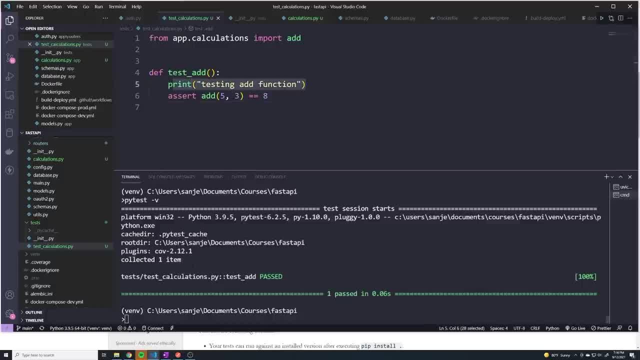 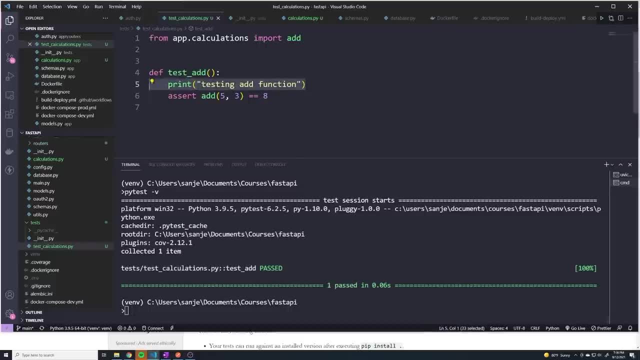 But nowhere in the output do we actually see anything get printed out. I don't see testing add function anywhere in here, And the reason for that is that by default, pi test will not actually print out any of your print statements. we have to pass in an extra flag to do that. 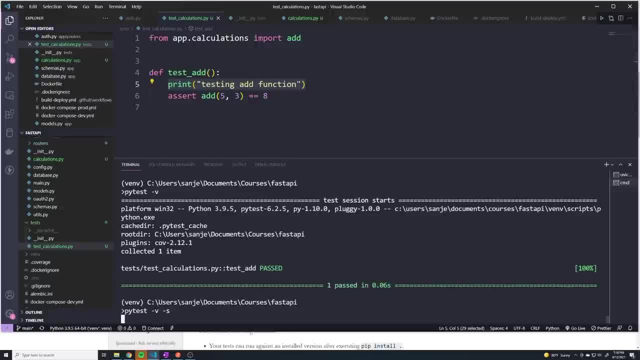 So to see the print statements you have to pass in dash s. So now if I run this, we can see that we ran this specifically Specific test and it ran testing add function And so keep in mind anytime you want to print something you got to pass in the dash s flag. 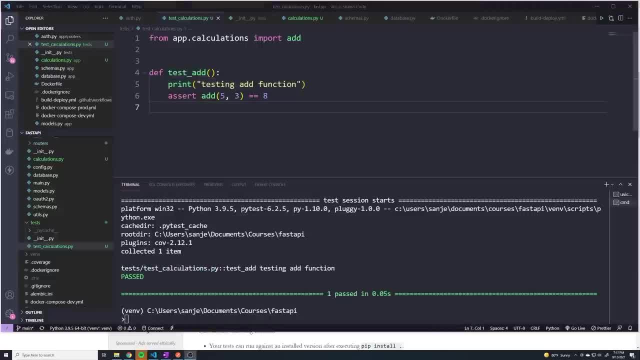 Okay, guys, so testing really is as simple as that. But before we go on to more complicated tests, I want to just make sure that we fully understand how this works. So we're going to create a few more dummy functions that we can use for testings. 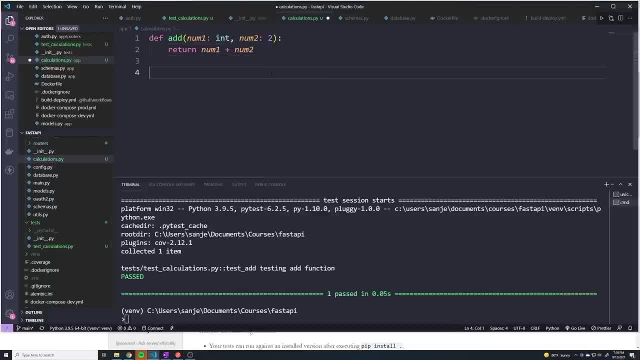 And if I go back to my calculations at py, I've already written this out, So I'm just going to paste it in here not to waste your time. But you'll see that they all essentially do the same exact thing. They just perform some sort of mathematical operation. 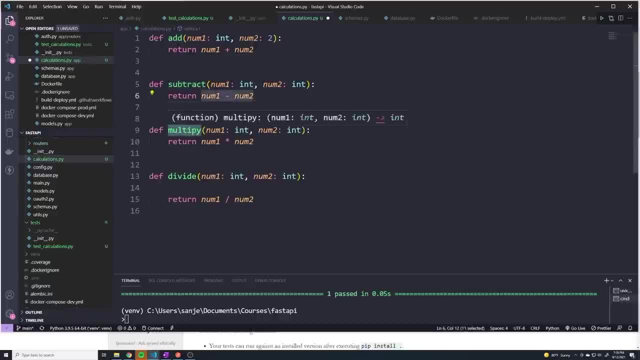 So I've got the subtract function, which just subtracts two numbers, I've got the multiply, which adds two numbers, and I've got the divide, which just divides two numbers. So let's test this out Now. The first thing that we got to do is, well, let's import all of those. 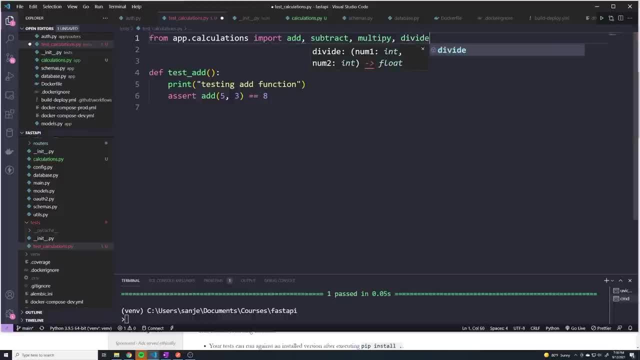 So there's subtract, multiply and divide, And let's define our function for subtracting, Alright, and so, just like before, I'm just I'm going to do a one liner, So I'm just gonna say assert and we'll say subtract two numbers. 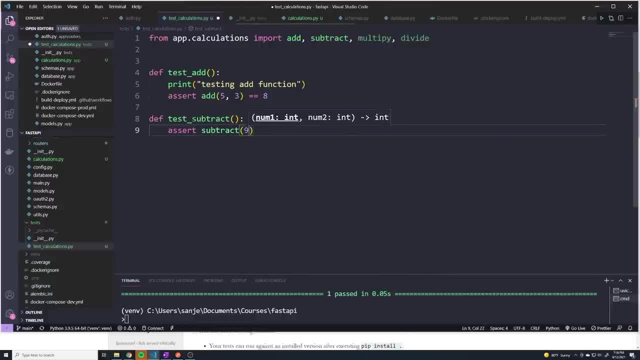 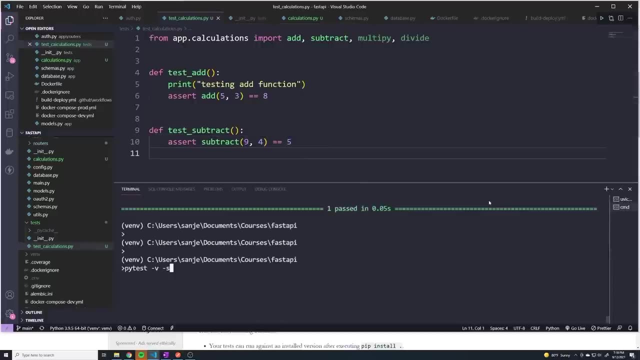 What numbers do I want to subtract? How about nine and four? oops, nine comma four. and we know that nine minus four should equal five. So I can do: assert equals equals five. Alright, and if I run this again, right, we can see. 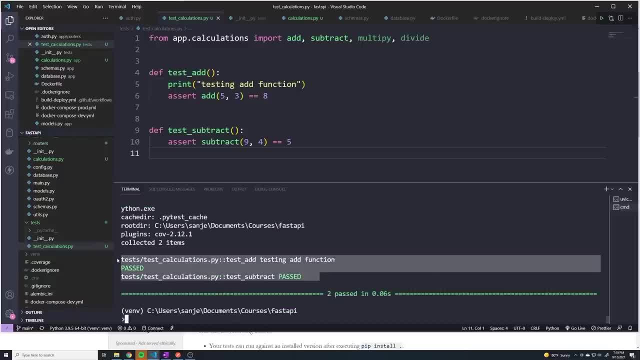 that both tests pass. And just to make sure that you know our testing actually works, Let's actually go into our code And let's essentially create a bug. So if I want to add two numbers, right, we know that it's gonna be num one plus num two. 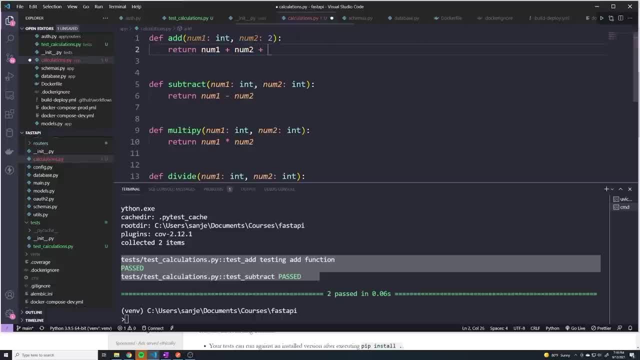 But let's say, you know, one of our moron colleagues went in and added one which is ultimately going to cause our function to break, And so ideally, if everything works fine in our testing, it should be able to catch this. 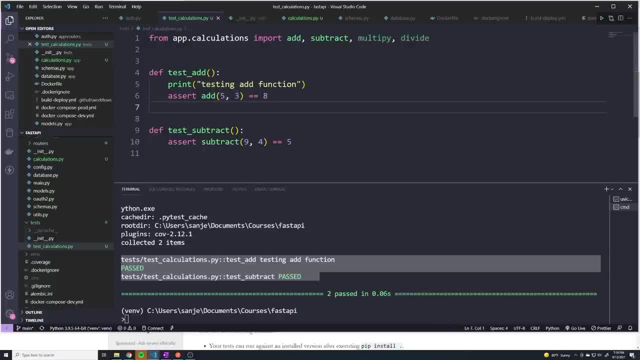 Because if we add five plus three, it's going to do five plus three, and then it's going to add that extra one. it's going to return 99. equals equals eight is going to assert to a false, which is going to throw an error. 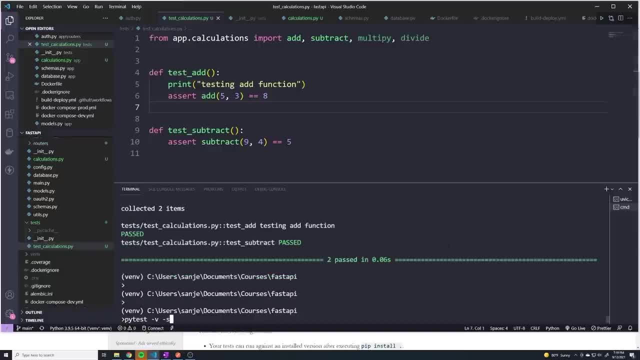 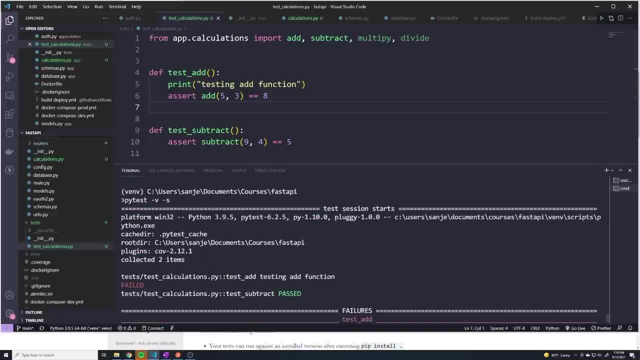 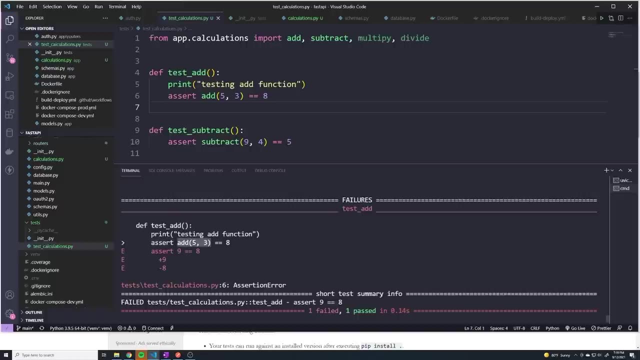 So if we try this out now, we can see that it did in fact fail And because we set this to be verbose, we can see exactly what happened. So we ran the test ad And what happened was it asserted: add five comma three equals equals eight. 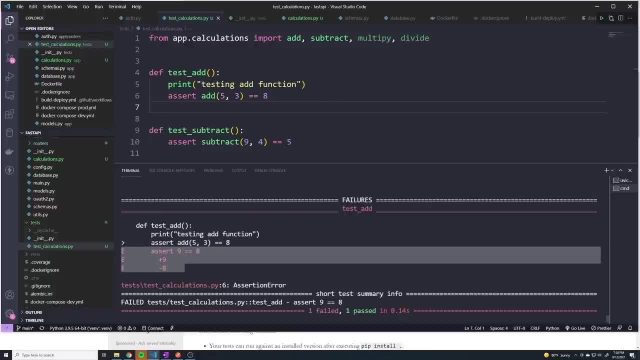 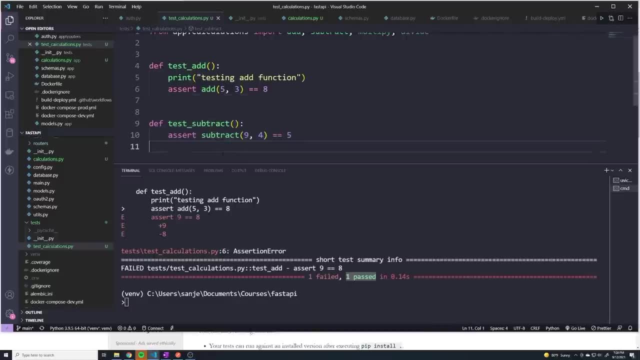 So it's asserting: nine equals eight and that's going to throw an error. And so that way we see one failed, one pass of the subtract function still passed because we didn't touch the code for that. So I'm going to go back and fix our bug in this case. 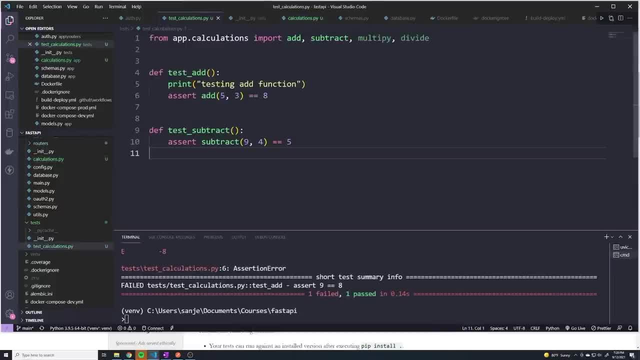 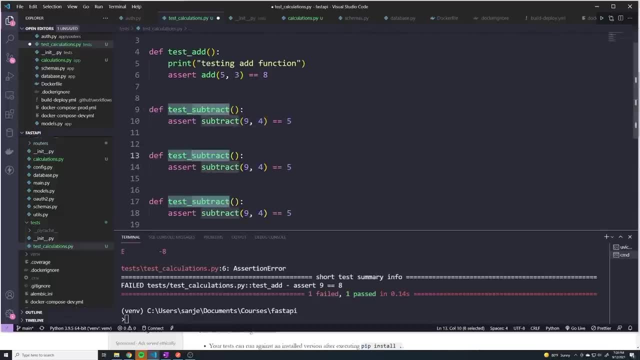 And we're going to just set up a couple more test functions for multiplying divide And I can just really just copy these. actually, I'll just change this to multiply divide And we'll just select a couple of numbers. So let's say: 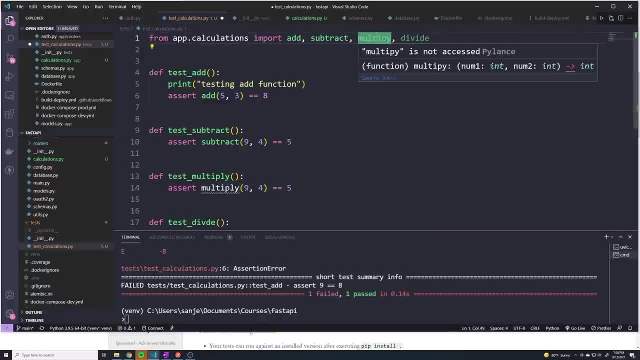 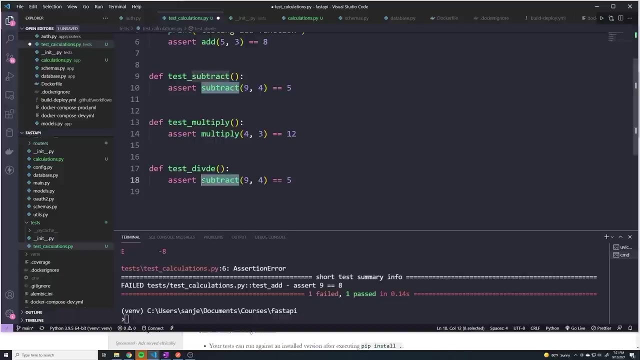 and I realized looks like that's a typo. this should be multiply with an L. All right, and we'll say four and three. when we multiply four times three, that should equal 12.. And for divide, we'll change the function that we're calling to be divide. 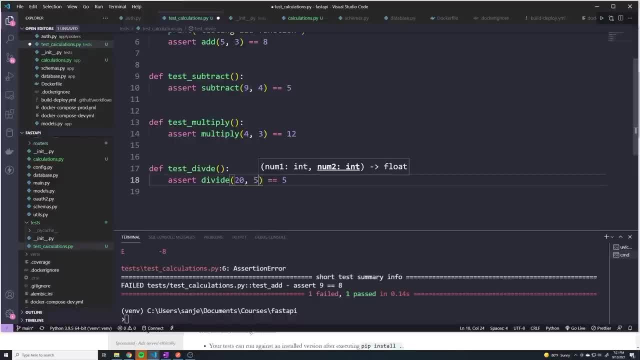 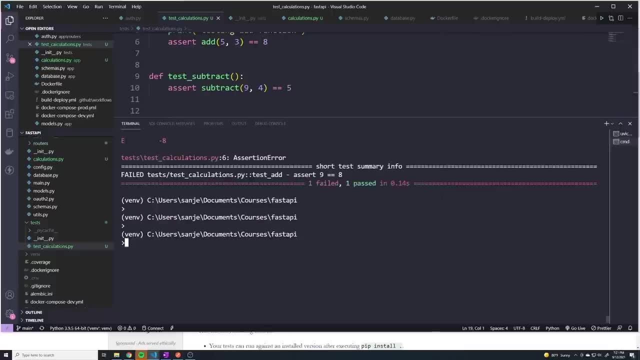 And we'll do 20.. Five, So 20 divided by five should equal four, And so now, if I save everything, we should ideally see all four of our tests pass. Let's try this out again, And you don't have to use the dash v or the dash s, like if you're not printing anything. 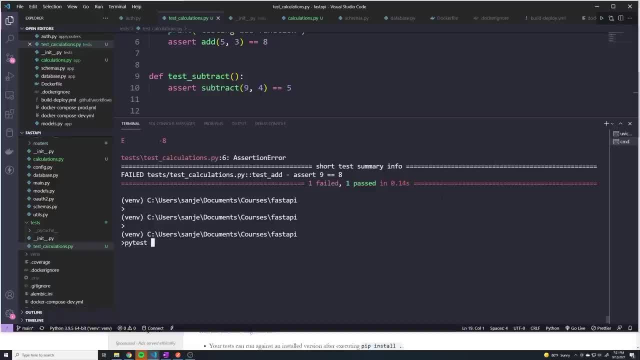 or you don't want to see it, you don't need the dash s And maybe you don't want the verbosity, So you can technically remove those as well And we can see that we get four dots, which means all four of our test functions have. 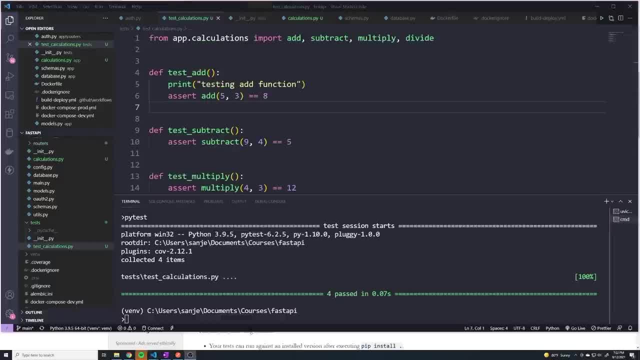 succeeded. If you're like me, the first thing that you may have noticed is that, you know, testing with one set of numbers Just doesn't seem ultra reliable, right? That doesn't necessarily assure us that the function that we wrote actually does what. 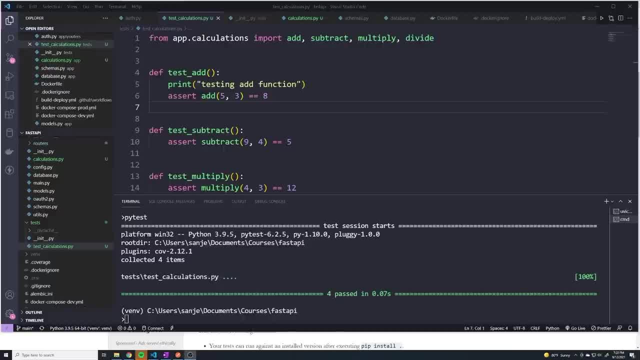 it's supposed to do. I would ideally like to test with a couple of different sets of numbers, And the way to do that is well, you know, I'm sure if you just took a guess right, you're probably thinking: well, maybe we just copy this function, paste it. well, that should. 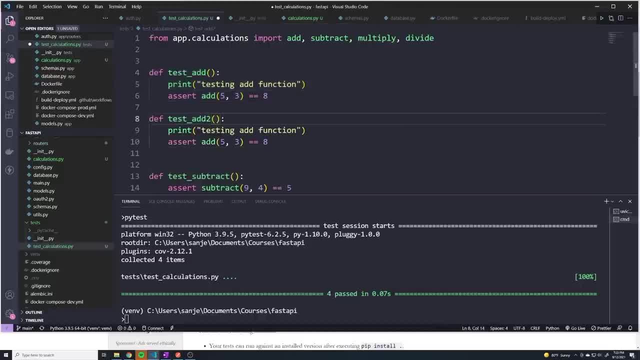 be back here And then maybe just call this test add to. maybe we don't need this print statement anymore. And then you provide the other sets of numbers, So maybe like four and two should equal six, And then you try this out. 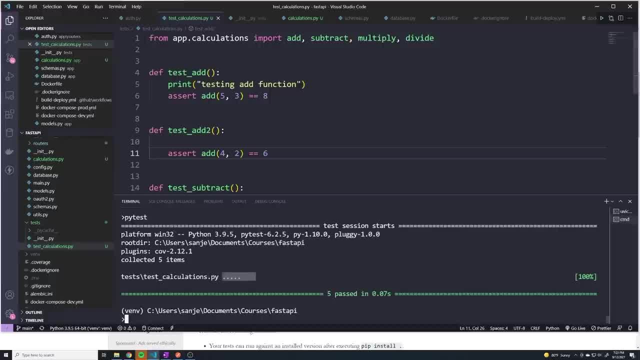 And you run this And we can see that that worked And technically you can do that. But pi test provides us a simpler way of doing this, So I'm going to delete this because we don't need that. I'm going to show you how we can do this using something called parameterize. 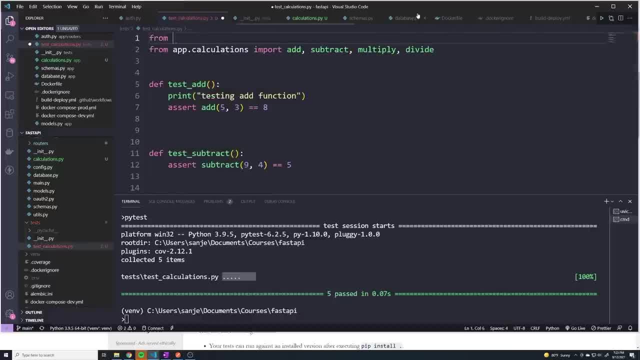 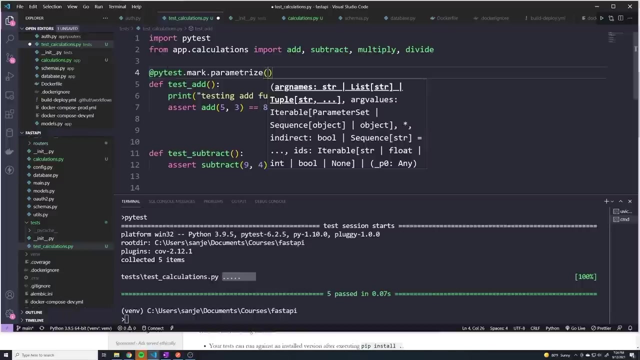 So I'm going to import pi test. So I'll say from. I shall just say import pi test. And we're going to add a special decorator from the pi test library. So we say at pi test, dot, mark, dot, parameterize. And so here we can essentially provide a list of numbers that we want to use for testing. 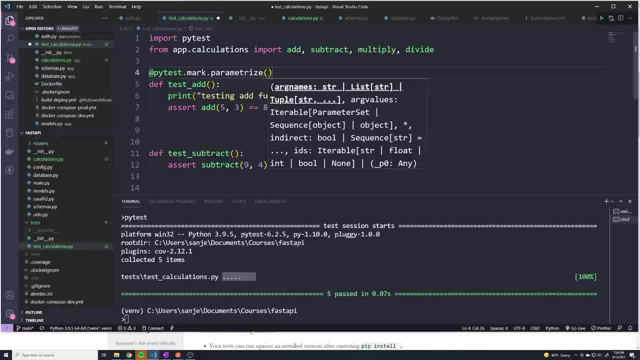 and then provide what is the expected result. And so you know, our function takes two inputs, five and three, And we also need to provide what is the result. So these are all the values that we're providing. We have three values. We have a specific function. 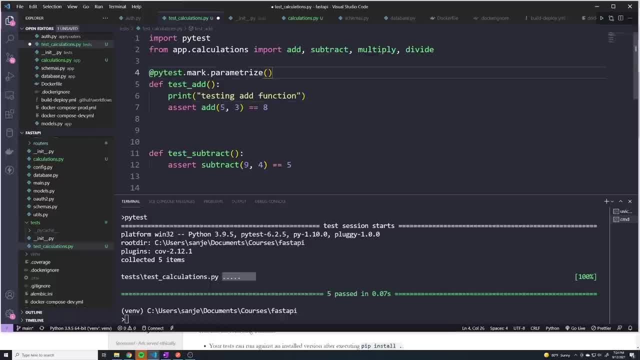 So we're going to tell this specific decorator what are the three things that we want to provide for each test case. So in quotations we'll do num one, num two and then the expected value. Now, what you call these doesn't matter. 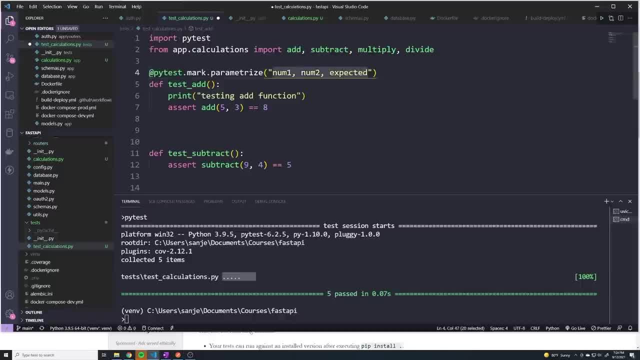 It's up to you, Right, But these are going to be treated like variables, essentially, So you can call them what you, whatever you want. You can call this x, you can call this y, You could call this, You could call this result. 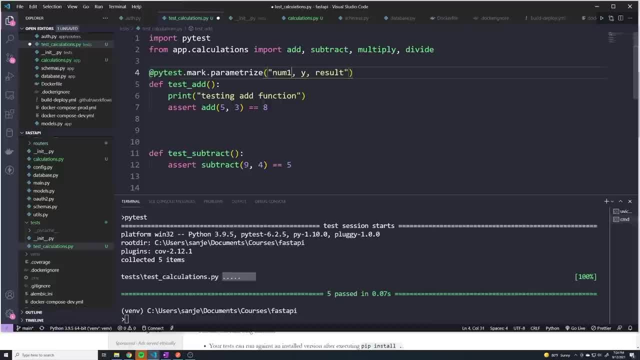 It doesn't really matter, But I'm going to stick with num one, num two and expected And, more importantly, take a look at how this is set up right. Your instinct is probably to do the end, quote here and then quote here, quote here and. 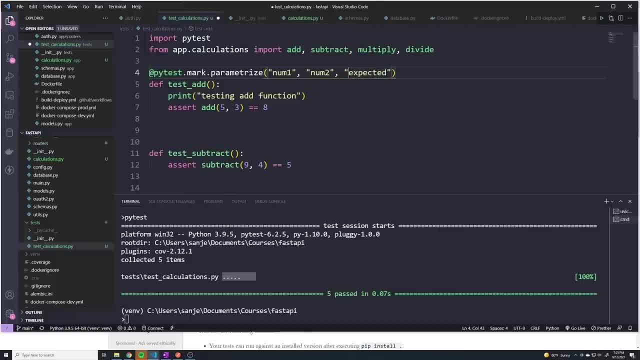 then quote here like that: That's not what we want, That is not how it actually works, which I don't know why they decided to do like this, but that's just what they've chosen. So instead, you remove these And everything should just be one big string. 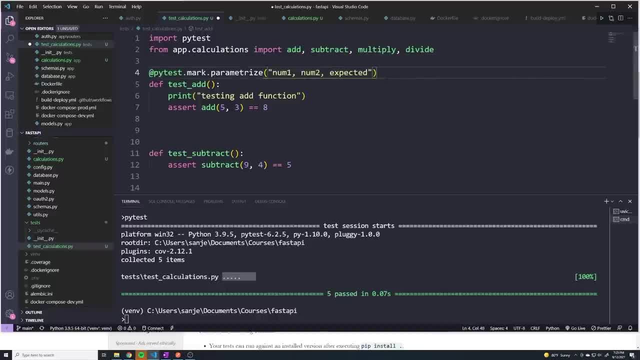 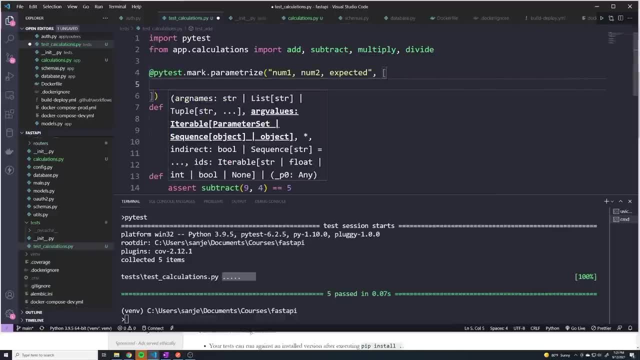 So that's the first argument into this decorator. The second thing is going to be a list and it's going to be a list of tuples and each tuple should represent one specific test case. So the first tuple, we're going to provide our test case values. 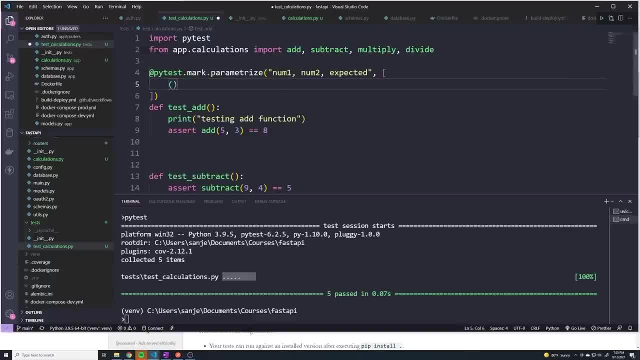 So we want, what is the value of num one? So in the first test let's say we want three for num one. What's the second one? that's going to be num two, so it's going to line up with what we've. 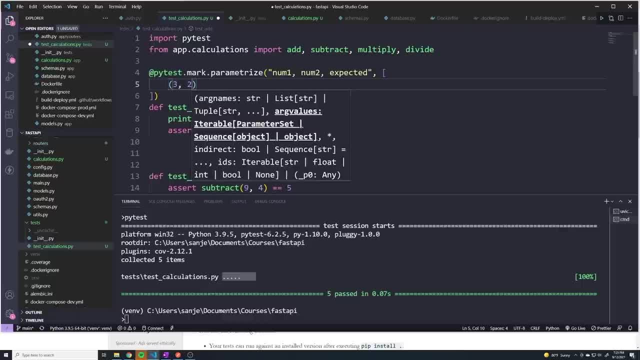 put here. So we'll say three, two, And then what is going to be the expected value? Well, three plus two should equal five. So we just say five, And so that's our first test. we want to add a second test? just do comma, add another. 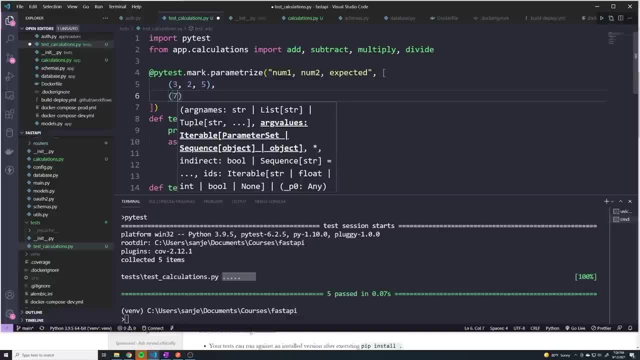 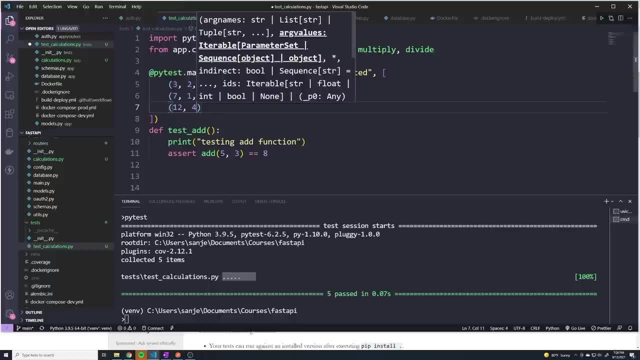 tuple And let's just add another set of numbers. So let's say num one is seven, num two is one. we know that should equal eight. And just one more test, And here I'll say 12.. Okay, And four should give us 16.. 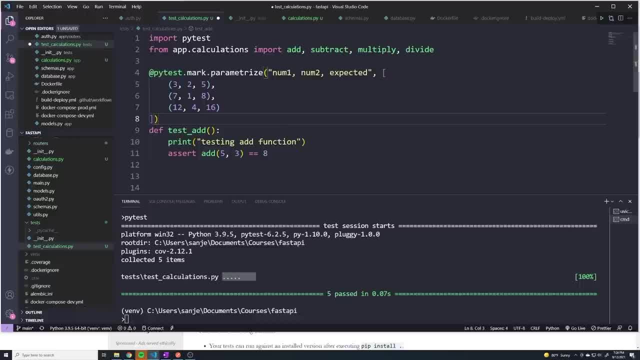 All right, And so now what we can do is we can pass these variable names into our test underscore add function. So I'll say num one, num two and expected right? so you want to make sure these match up with what you've placed here. 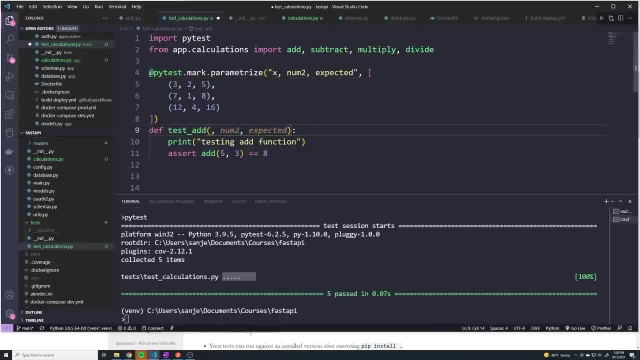 Because if this was called x, then you want to make sure that this is called x. But we'll change that back. And now, in our context, we're going to add another test, our code. we want to replace all of our test values with these variables. So this is going. 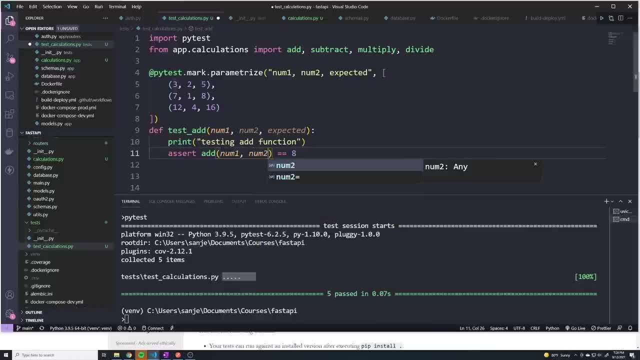 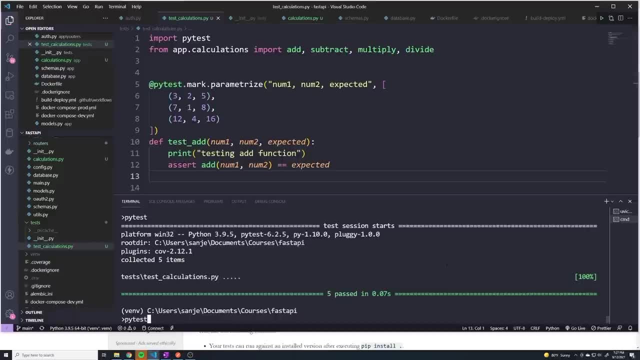 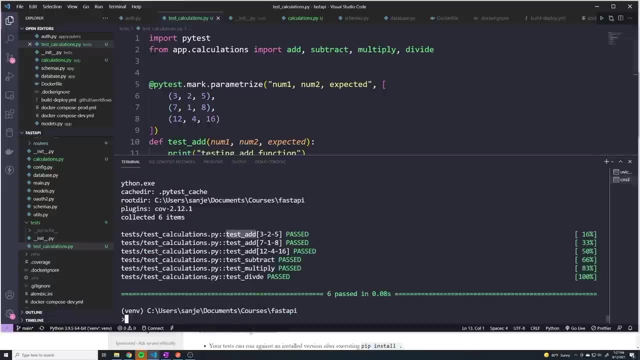 to be num one, this is going to be num two and this is going to be expected. And so now, if I run this and we'll just do a dash V just to see it more in detail, what's happening, Take a look at what's happening Now. we can see that test ad ran and it ran with 325,. 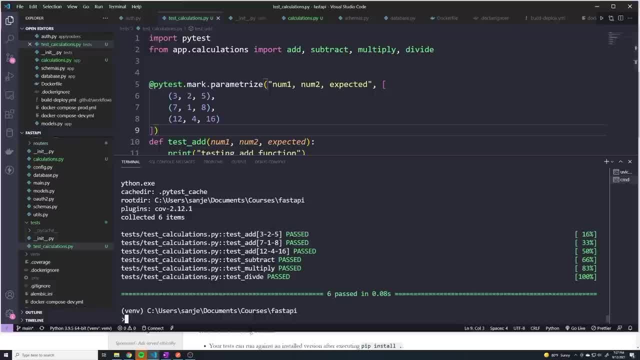 which is the first test case it passed. then it ran the same exact test with these values- 718. that passed. and then it ran with these values And that ran, And it passed just fine. And then finally, all of the other functions also passed as well. So this is one way of. 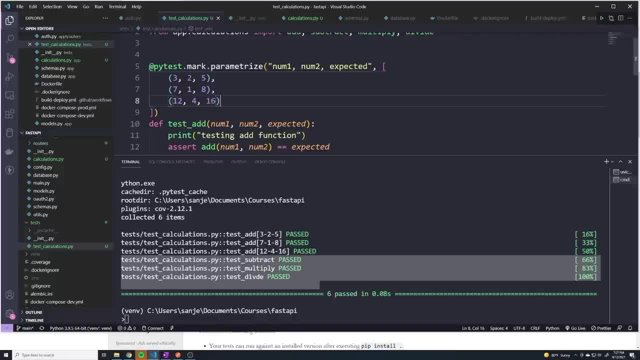 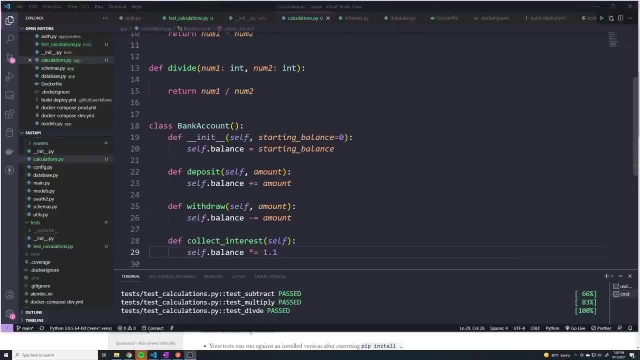 running the same test over with multiple values without having to just define 345 functions and just copying and pasting. It's a little bit cleaner doing it like this. So till now we've just tested some simple functions And you'll see that when it comes to testing, 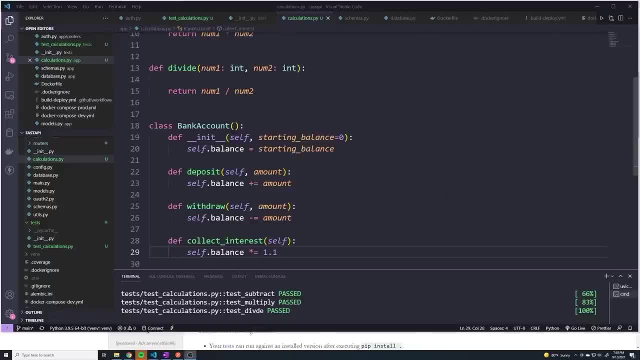 anytime you want to test a function. it's actually pretty easy. However, when you're working with classes, it gets a little bit trickier and it usually involves having to write a little bit more code. So I've created a simple dummy class, in this case called bank account, And this: 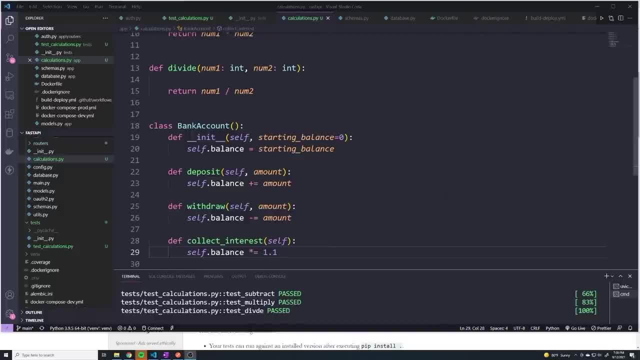 represents a person's bank account And I've already written this out because I didn't want to waste your time writing this out. So if you want to pause this video and just copy down the code so you can follow along, go ahead and do that. But let me just quickly. 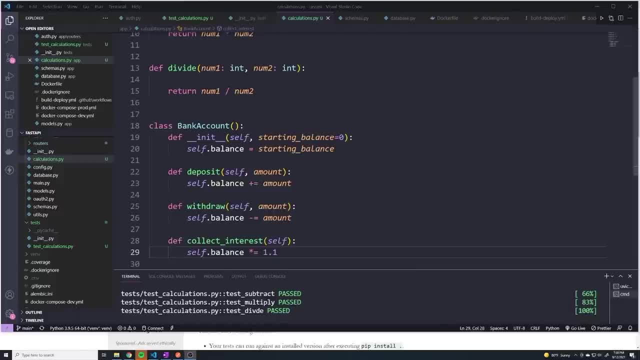 walk you through what this specific class is doing. But, like I said, this represents a bank account. So first of all we've got the constructor. So when we create a bank account, we create a bank account with a specific amount of money which is going to be referenced. 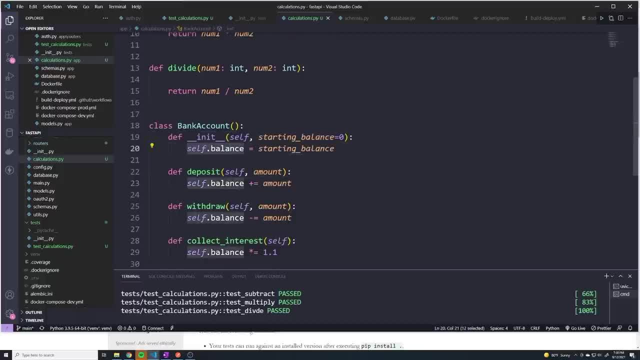 by the starting balance value And then it's just going to set the balance property of the bank account class to be whatever you provide. If you don't provide a starting value, it's going to default to a value of zero. Then we've got three different methods. We've 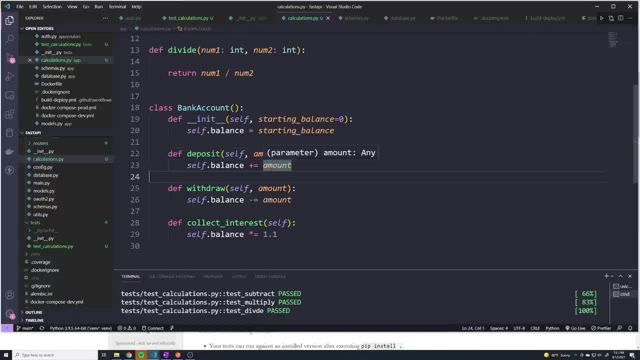 got Deposit, which means we're going to deposit money into our bank account. So all we're doing is we're going to pass in a value And then we're just going to add it to our total balance. Withdraw is the opposite: We're going to subtract a certain amount from our 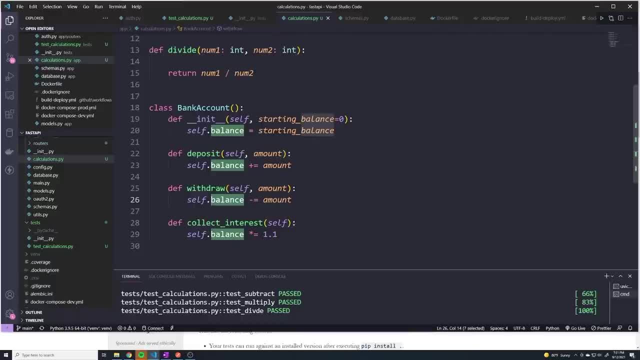 balance. And then interest is simple: we're just collecting interest. So here we just take our balance and then multiply it by 1.1, which I guess would represent a 1% interest rate. And so those are the three or four functions methods, if you want to count the constructor method as well. 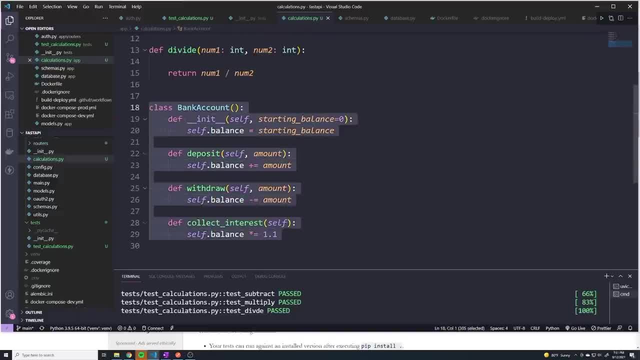 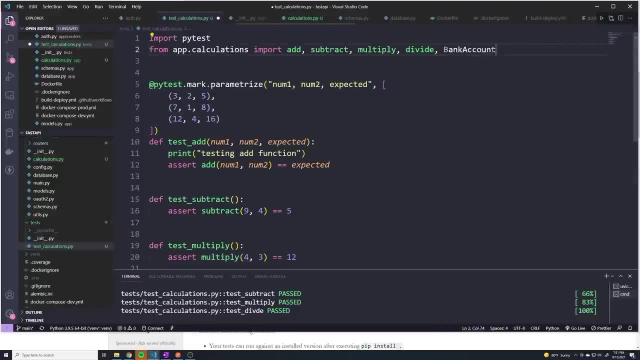 that our bank account class has. So I want to go ahead and test this out now. So we'll go to our test calculations And, first of all, we want to import our bank account class. So let's create a test for our bank account. 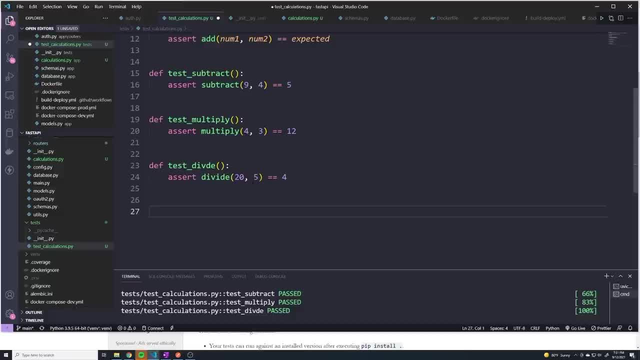 And the first thing I want to test is: let's create a brand new bank account where we set the default value, the initial amount, to be 50.. So here I'll say test, And I'm just going to call this: maybe test bank set initial amount. I want this to be as 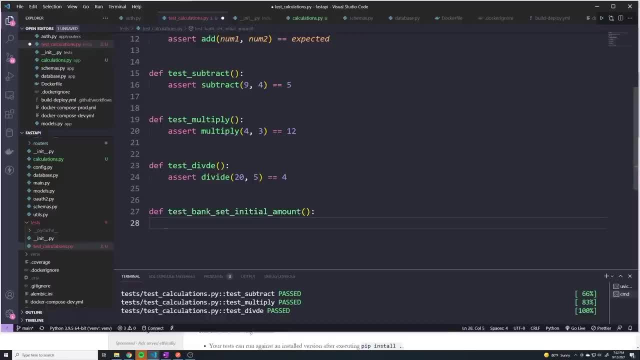 descriptive as possible. So I'm going to say: test bank set initial amount. I want this to be as descriptive as possible. And so here, what we're going to do is, first of all, we're going to create a brand new bank account instance And, since this test is going to test to ensure that 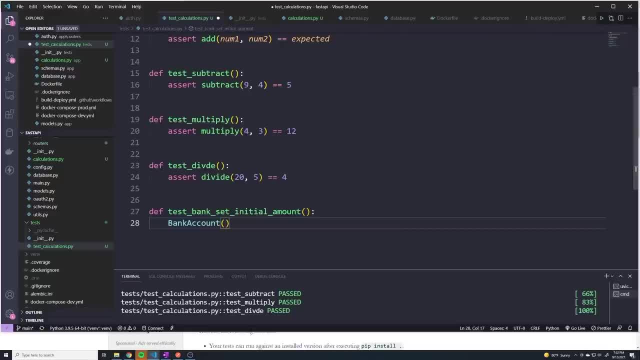 we have actually created a brand new bank account with a certain amount of money. I'm going to provide a value, doesn't matter what value you decide to use, but I'm going to use 50. And we'll just store this in a variable called bank account. All right, and so to test if 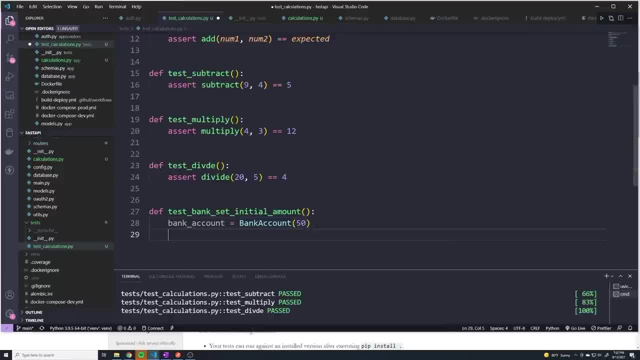 if our function actually worked or the functionality of our constructor method actually worked. what we're going to do is we just say assert And we want to check the bank account dot balance property equals equals 50, because we set the default value to be 50. And if we just 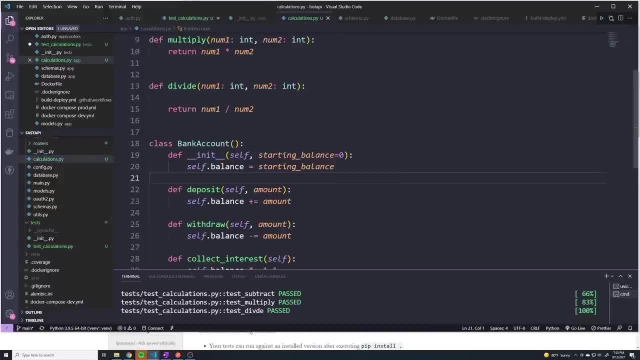 quickly go back to our code. you can see that we set the starting balance or we set our balance property to be. whatever the starting balance is, it just happens to be a default of zero if we don't provide one, but we are providing one. So we're going to set the starting balance to be. 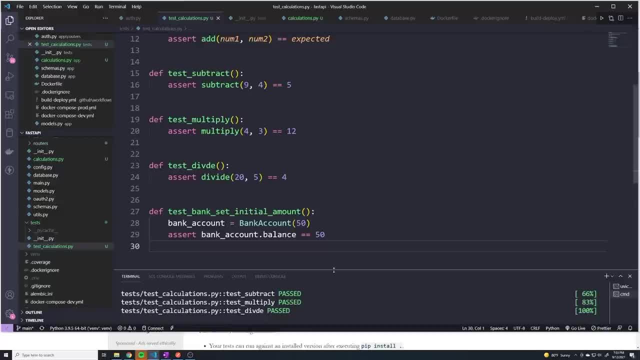 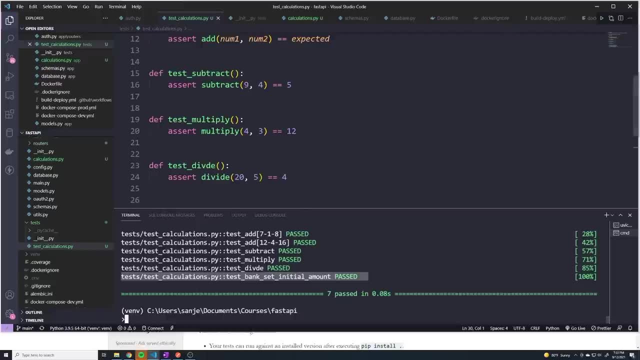 one, And that's what we're testing, So we can test this. Let's run our code now And let's see if this worked. We can see that it did in fact work, And just to introduce a bug, maybe we set starting. 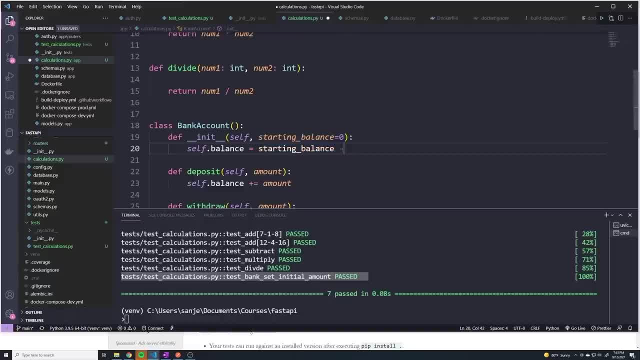 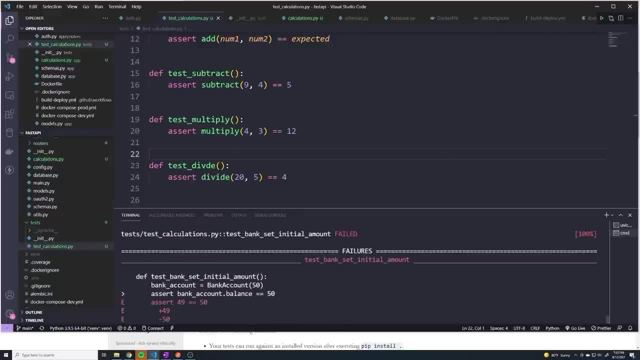 balance to be, you know, minus one, right. So we've broken our code. Now, if we run this one more time, right, you can see it failed because we subtracted one. So we're asserting: 49 equals equals 50, which throws an error. 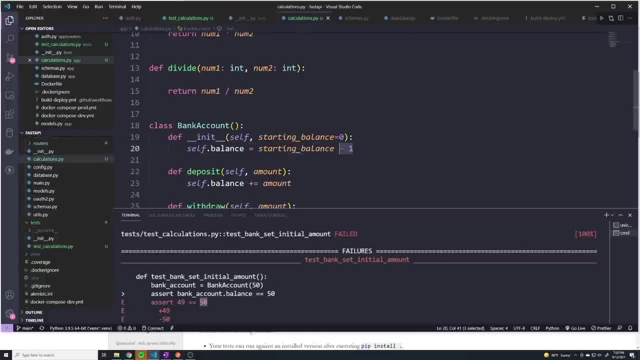 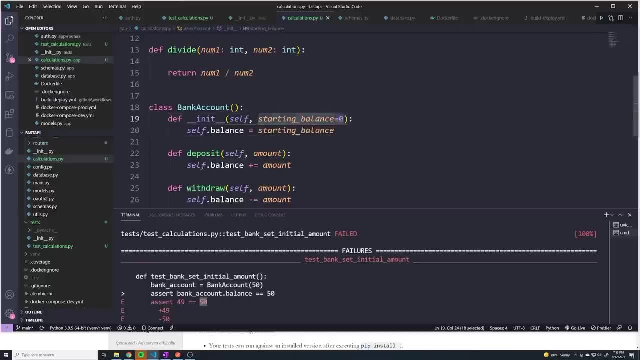 Which means we ultimately fail the test. Let me remove that bug. All right. the next thing that we want to do is: let's test to make sure that the default starting balance works as well. So I'm going to create another function And I'll call this about. 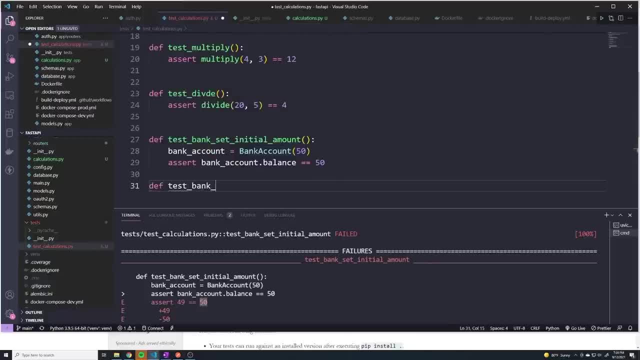 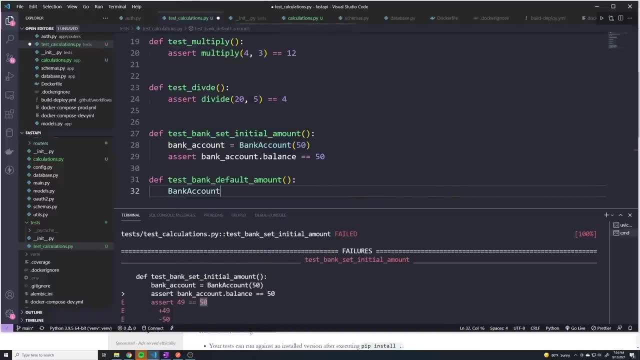 test bank underscore default amount. So in this case we're just going to create a brand new bank account And we're not going to pass in a value, So it should default to zero if Could, of Buy CodeWorks, And then we'll. 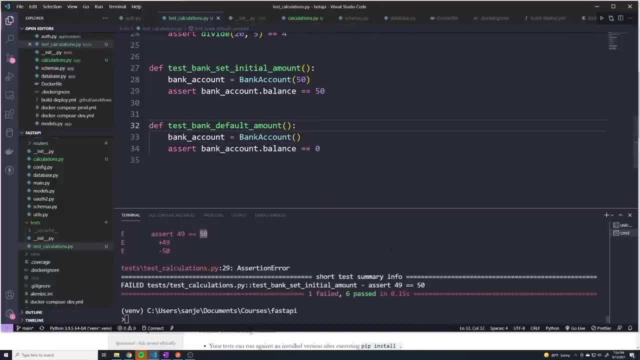 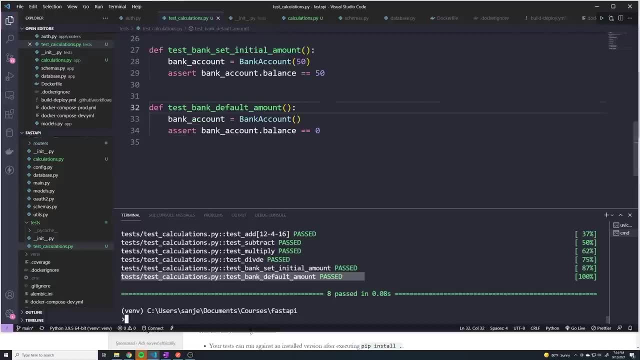 store this in a variable, just like we did before, And then we'll assert. I can copy this, But now it should equal zero. Okay, and let's test this out. now Looks like it works so great, And let's just quickly go ahead and test our last two functions out. 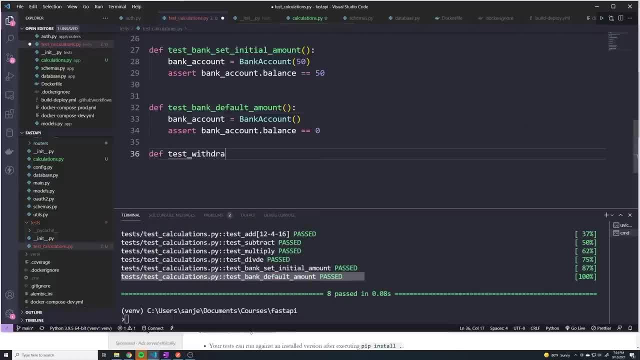 Sorry, we got withdrawing functionality, So I'll do test underscore withdraw. And here we're going to initialize another bank account instance. because we have to do that every time we want to test it, I'm going to give it a default value of 50. It doesn't have to be 50. Once. 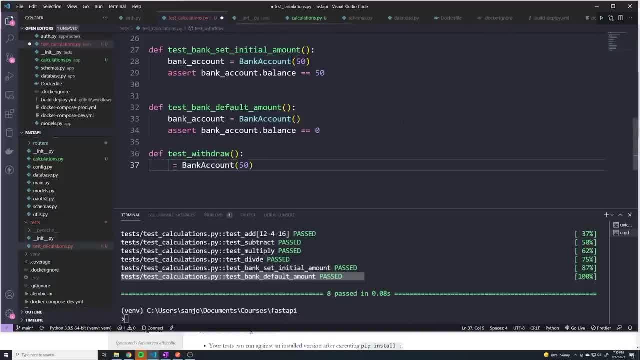 again, you can choose whatever number you want And we'll store that in a variable called bank account And we'll call the bank account withdraw method And we're going to withdraw, you know, let's say, $20.. So we start out with 50, we withdraw 20, we know that the result should be 30. 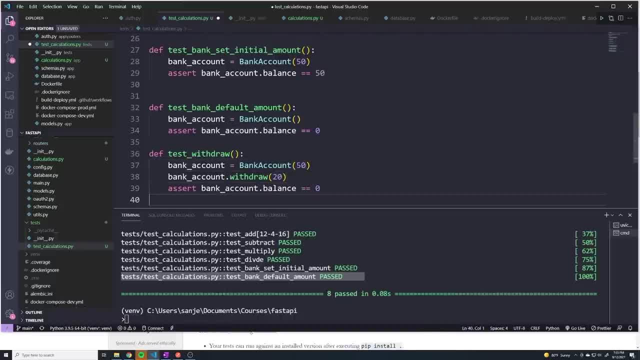 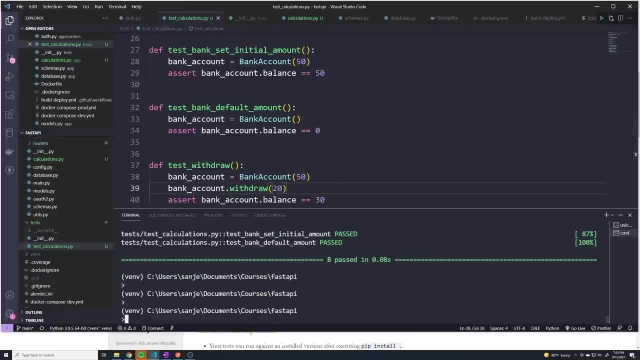 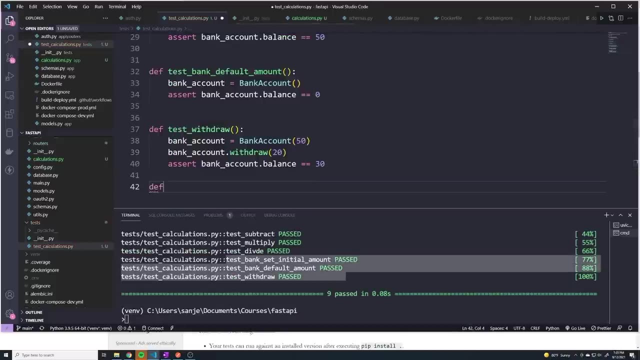 So if I just copy this assert statement once again, I can just change this to 30. And it should be no problem Run this Once again. all of our tests have passed. Let's try the deposit functionality Now. so I'll create a test to test that, And I'm actually just going to copy all of this. 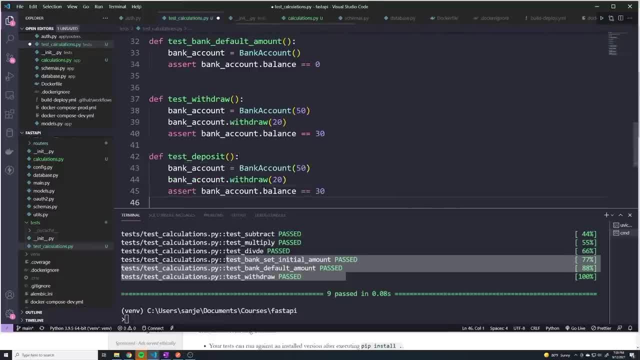 code because it's pretty much identical. You'll see that testing can become a little repetitive. We'll start out with an initial value of 50. doesn't really matter. We'll change the method to be deposit. Maybe we want to deposit $30.. So 50 plus 30 should equal 80.. We test this. 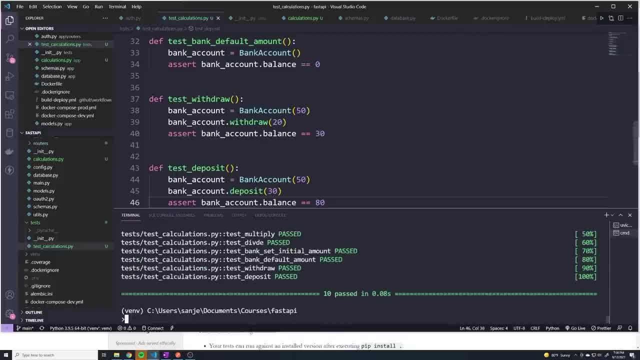 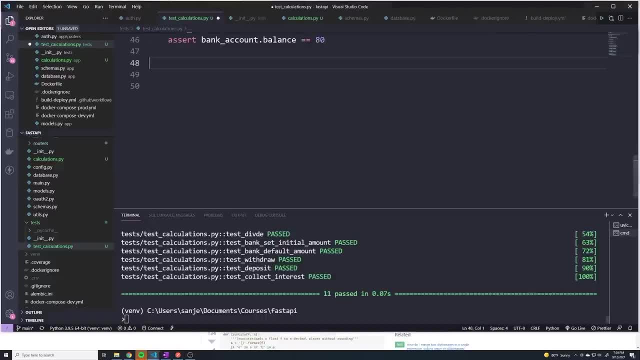 out Okay, Looks like everything's working, And the last thing that we want to test is the collect interest method. So let's create a function for that. We'll do test underscore collect, underscore interest And once again, I'm going to copy this code And we'll just use it here, which is going: 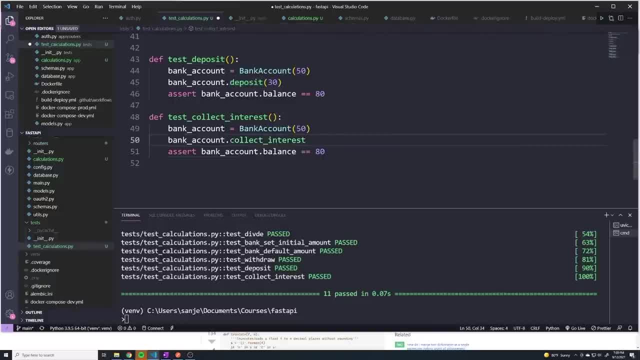 to change the method to interest. Okay, so we start out with the value of 50. And so what should the interest be? What? if I take a look at what my method actually does? it just takes the number, multiplies one point. 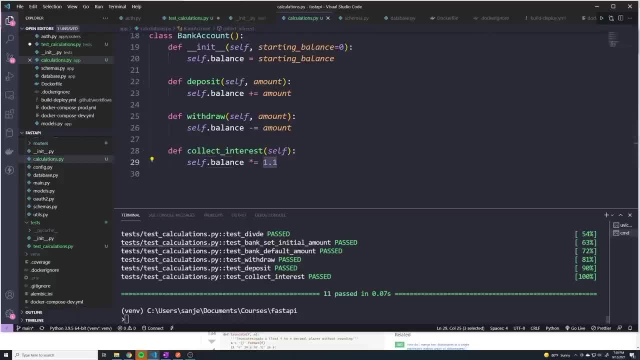 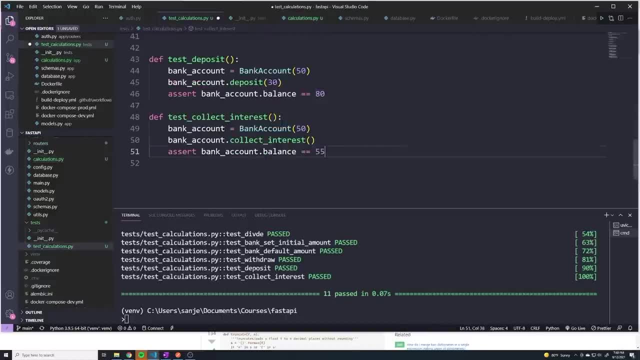 one. So that should give us 55,. right, 1.1 times 50, should be 55. So I will say this should be 55. And let's see what happens. So if I run this, we can see that we did have. 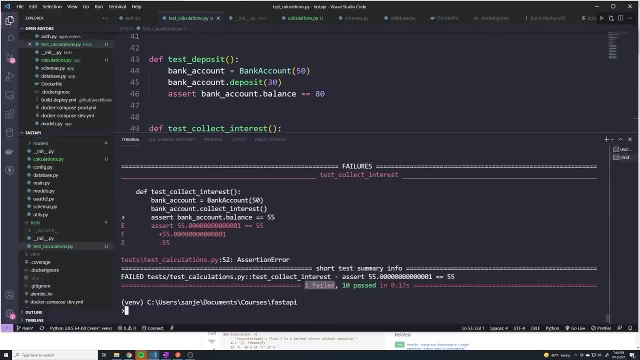 have one test failed- And I'm assuming it's going to be the last test, the one we just created- And we can see that the test collect underscore interest failed And the reason for that is that looks like bank account dot balance returns a value of 55.0000001, which in Python is not the 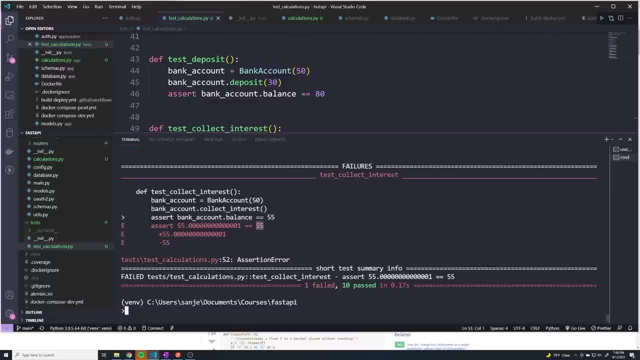 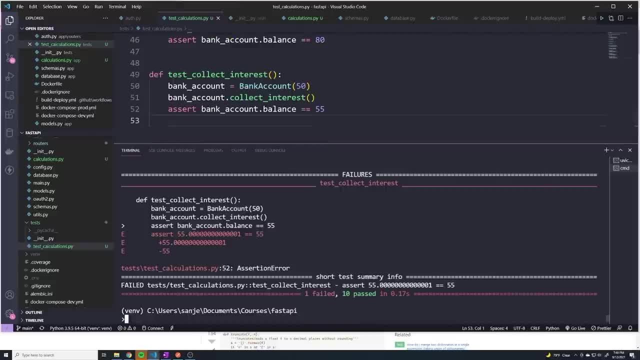 same thing as 55. So this isn't necessarily an issue with our code. It's just the way that you know. we're comparing numbers in our test. So this is an issue with our test in this case because it's not accounting for some of the different rounding and the way that calculations 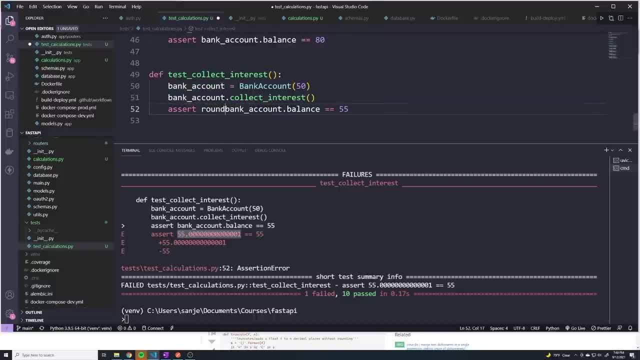 occur within Python. So what we're going to do is we can just call the round method right here and we can round it to you know five or six decimal places, depending on how accurate you want it to be. So it should now round it to you know. this value, however many decimals, is five. 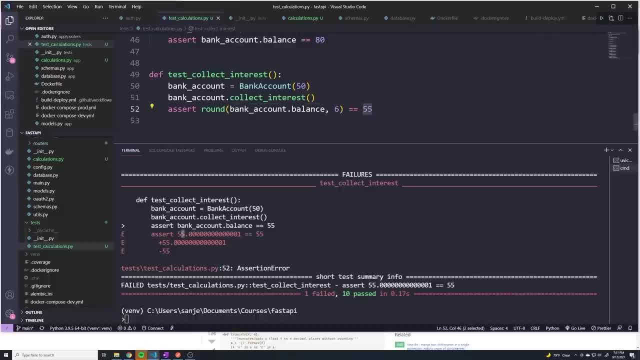 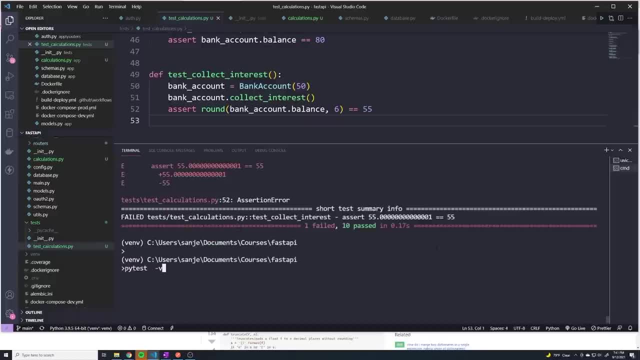 or six, and then convert it to an integer. So then we can compare these two, because this is an integer, this is technically a float, So not exactly. they're not going to be equal in that case. So now, if I run this, 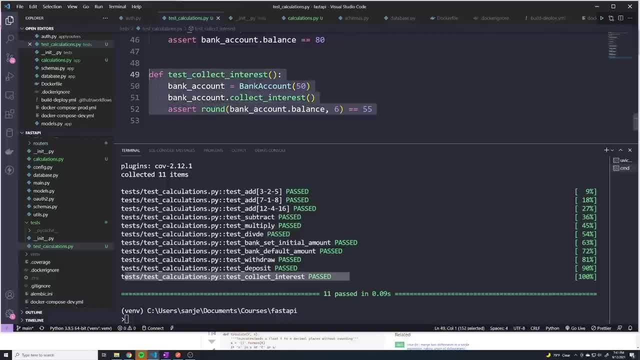 we can see that it did successfully pass. So that's just something to keep in mind. That's why I added that little extra test case, just to make sure that, especially when it comes to those calculations, you got to make sure that you're comparing the right two numbers. 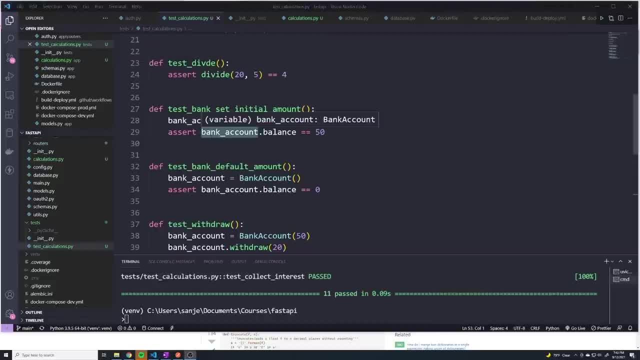 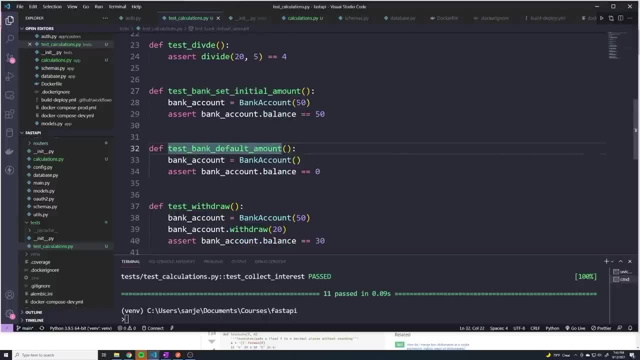 If you look through all of the test cases for the bank account, you'll notice that there's some repetitive code right For every single test case that we have for testing our bank account. you'll notice that we always have to initialize a bank account instance. 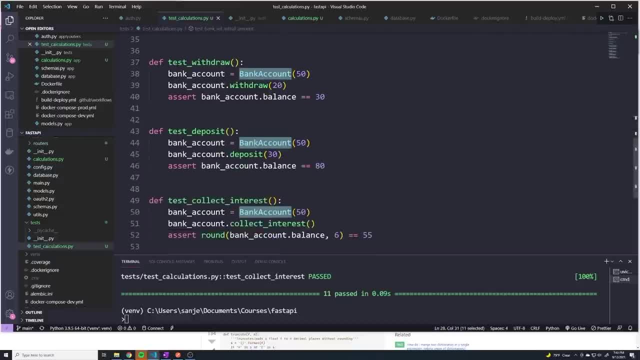 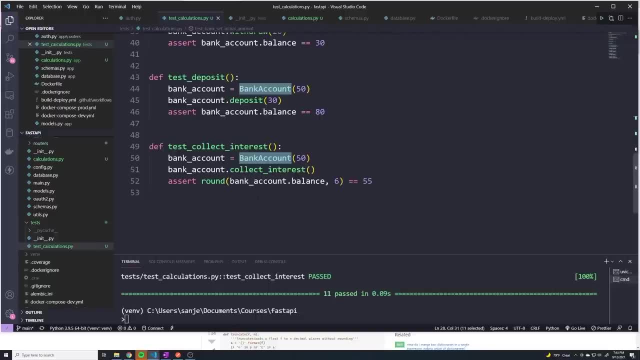 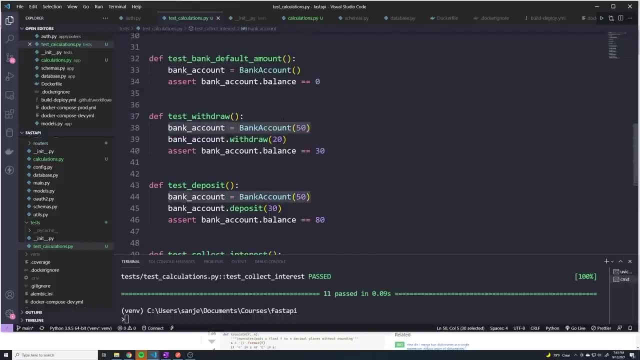 And you can see that right now. look at that we are repeating our code across all of our tests. And when you get to more complex classes, more complex test case scenarios, you might have 50 tests for a single class And we're, in this case, just repeating the same exact code for each one of them. And so when 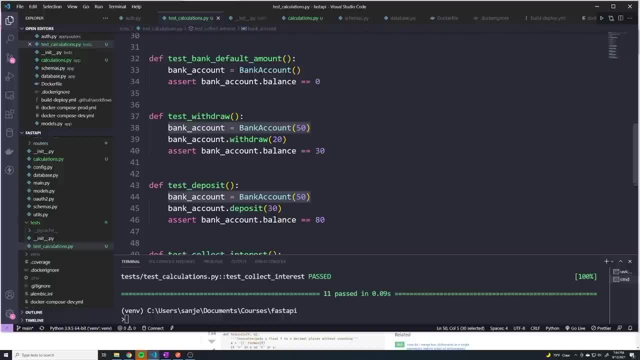 it comes to writing these tests. you know, pi test does provide us with some tools that we can use to minimize the amount of repetitive code, And one of those is called fixtures. And a fixture is a very simple concept. It's an algorithm, It's an iterative tool, It's a standard, But it has to46: 00. 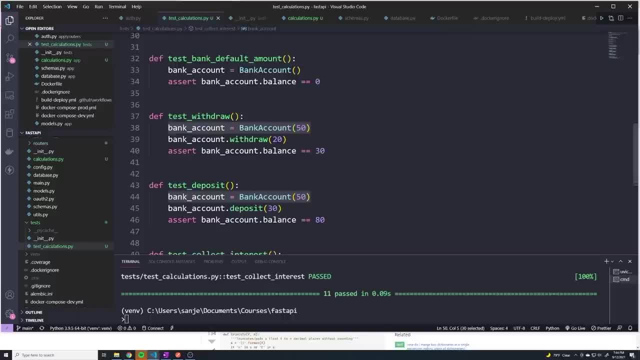 It's nothing more than a function that gets run before each one of your tests, or at least the specific test that you want. So we can create a function which does nothing more than initialize a bank account and then return it to our function. that's about to run. 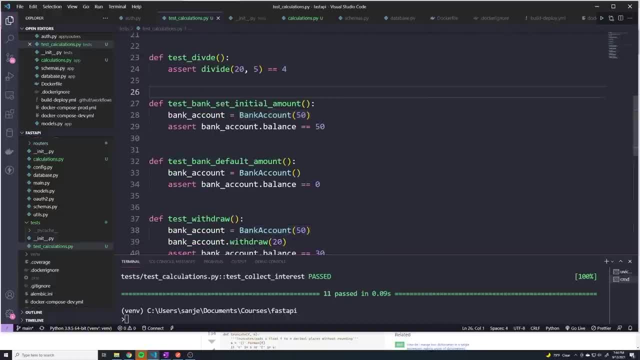 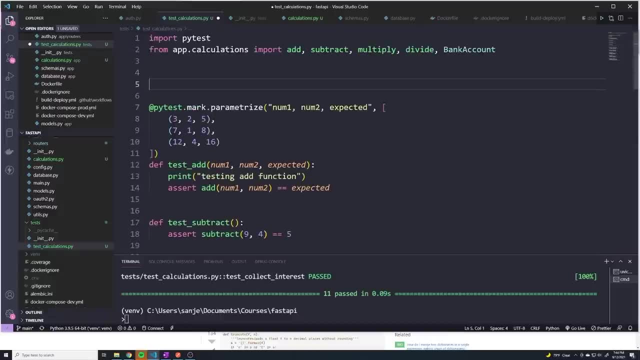 So I'll show you how we can do that. The first thing we have to do is let's create our fixture, and I'm going to. we can put it anywhere. I'm just gonna put it here for now, But generally you want to put it at the top of the file. actually, I'll stick to the best. 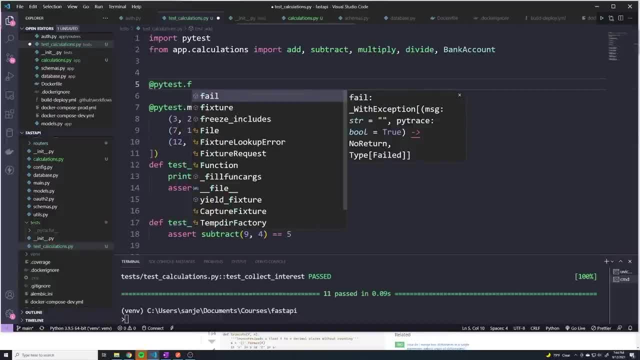 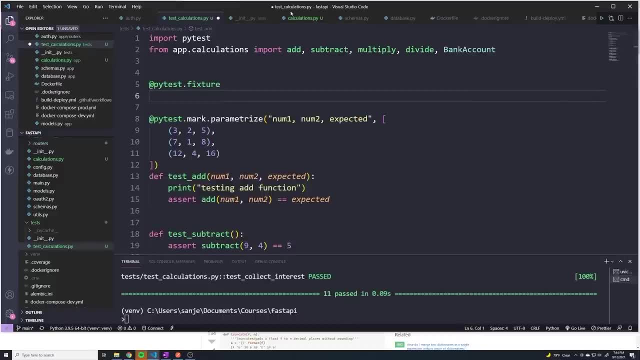 practice I'll say at pi test dot fixture, And then here we create a name for our fixture. So I'll say this is going to: you know, give us or initialize us a bank account with a zero initial value. So I'll call this zero underscore bank account. 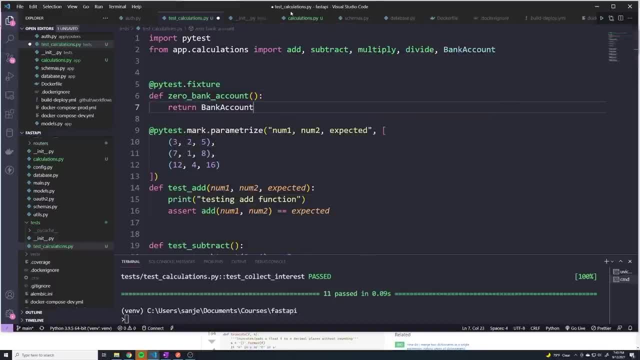 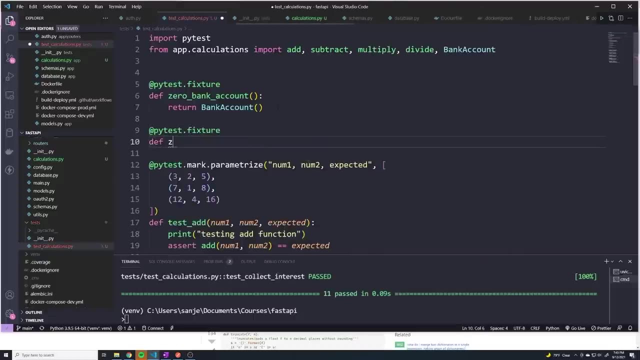 And so all we're going to do is we're just going to return an instance of bank account With an initial default value of zero, And then we'll create one more fixture, And this one is going to return a regular bank account with an initial value. and what? 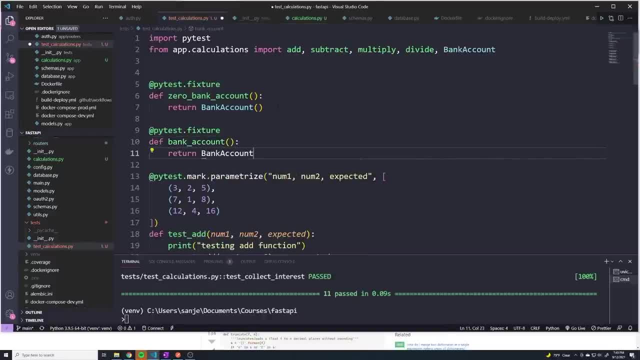 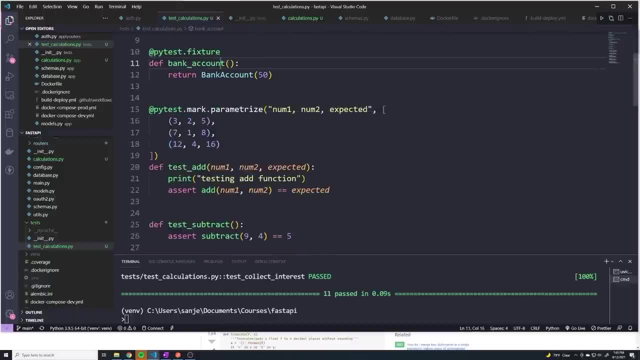 value we want to give it. we get to decide. So I'll just say return bank account And in this case 50. Alright, and so now what we can do is for all of these tests. I don't need to initialize. 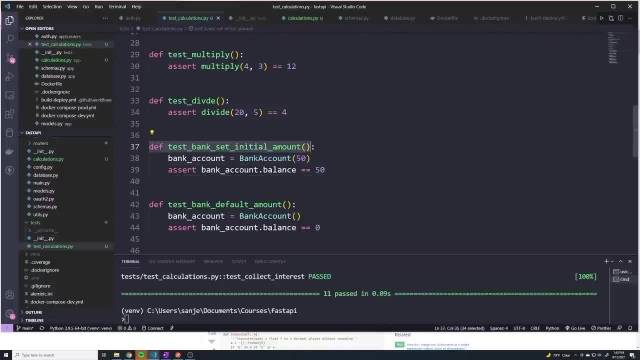 them here because I can have these guys reference the fixture. So to assign a fixture or have a fixture get called for, a function, we just pass it in as an argument. So for test bank account set initial amount, we're going to reference the zero underscore. 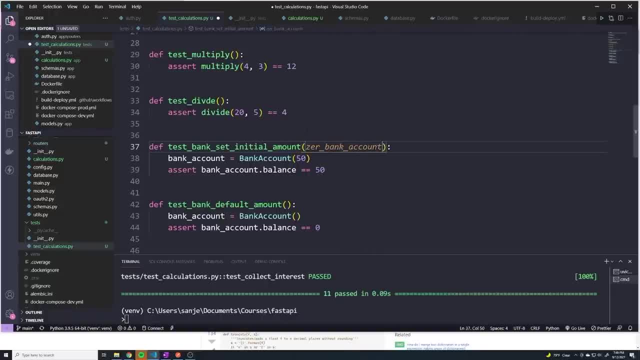 bank account fixture. So what exactly happens is when pi test goes to run this test case- because it sees this as an argument- into the function, it's going to- oops, that should be a zero, okay, But what it's going to do is it's going to call this function. 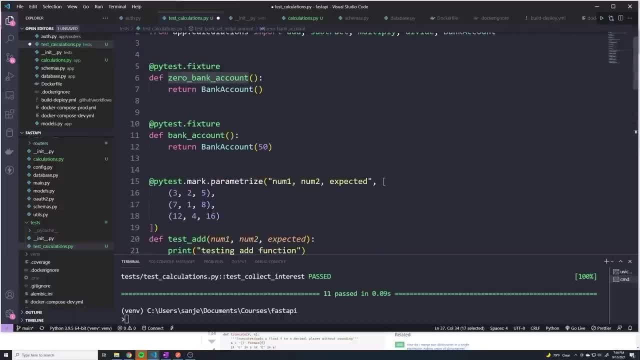 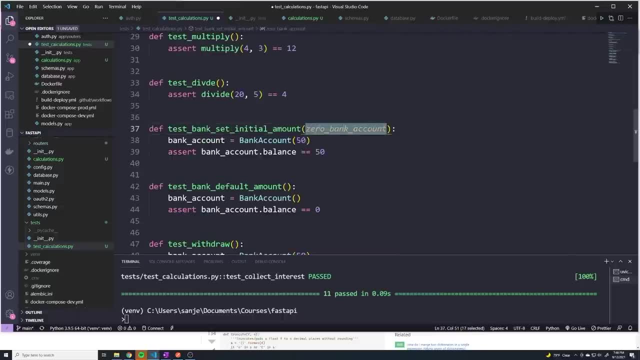 Before it actually runs the test case. So it calls this function And then whatever we return here, which is the bank account, gets passed into a variable called zero bank account. And so now, instead of creating a bank account instance, I can remove this. 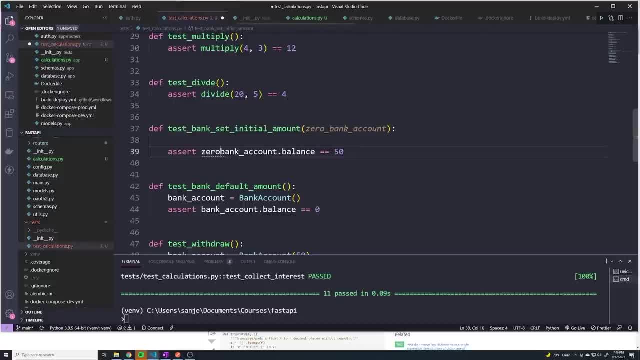 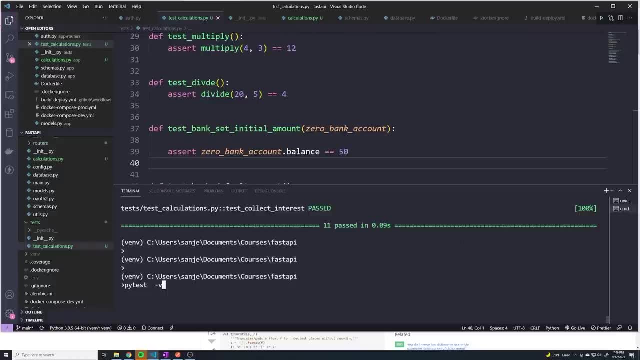 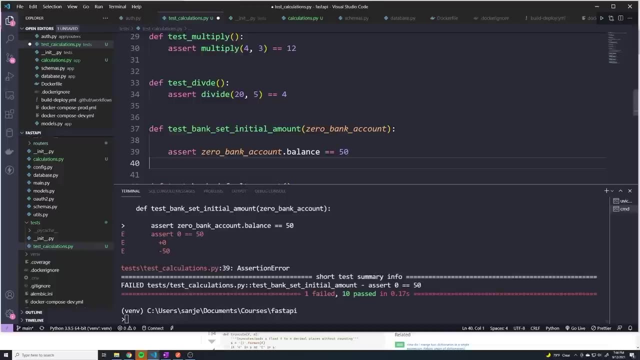 And I can reference this variable, which is zero underscore bank account. Let's test this out. Let's see if that broke anything If we run this. Oh, sorry guys, Let me undo this. I didn't mean to use this function. 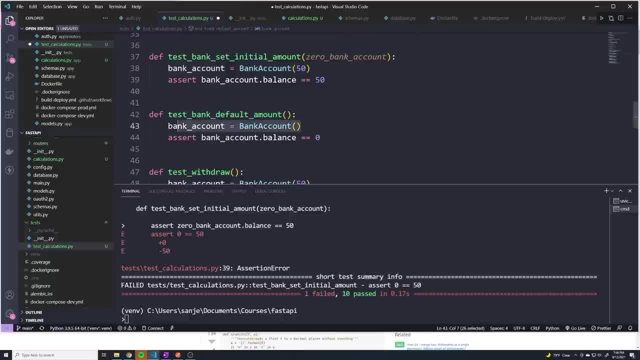 This is going to be the for the, the test bank account default amount. So we want to remove this one, my apologies, and we don't need that in this one. And then this will be zero underscore bank account. So now all tests should pass. 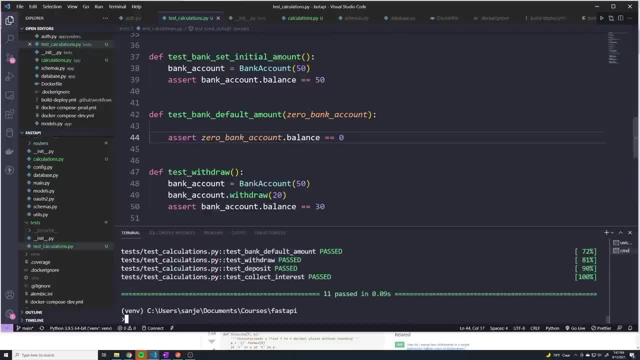 Alright, so everything passes. But if you're still a little confused as to the, you know what exactly does this mean? I'm going to go ahead and do that. I'm going to go ahead and do that. I don't know what exactly is happening behind the scenes or what is the order of operations. 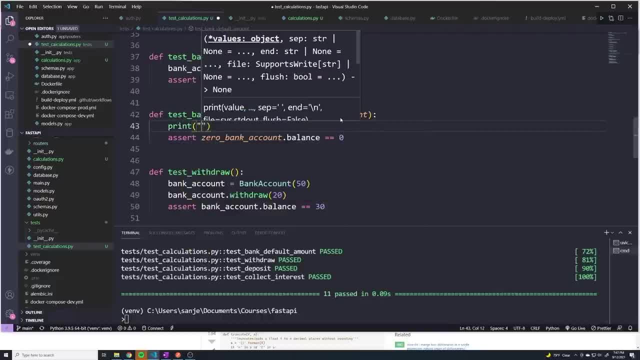 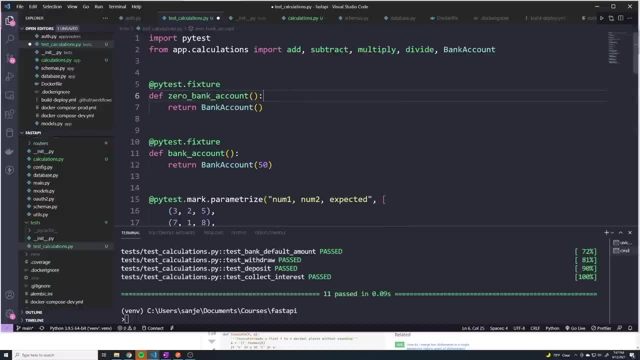 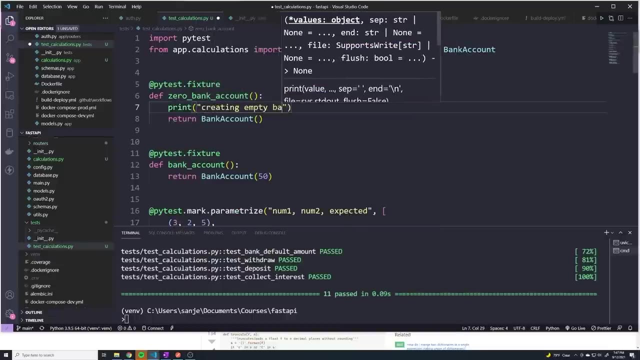 I'm going to add a few print statements. So I'm going to say testing my bank account, And then I'm going to put in a print statement inside my fixture as well, which is, say, creating empty bank account. And so now, if we run this, I want you to take a look at the code. 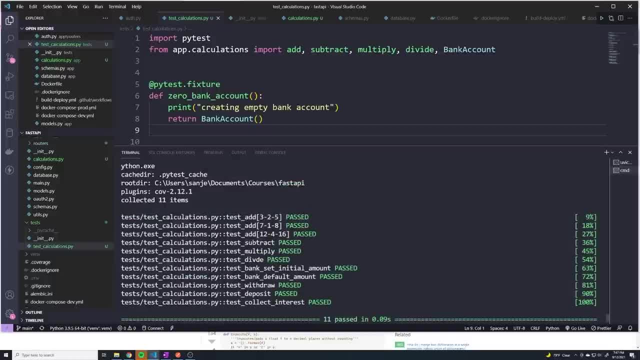 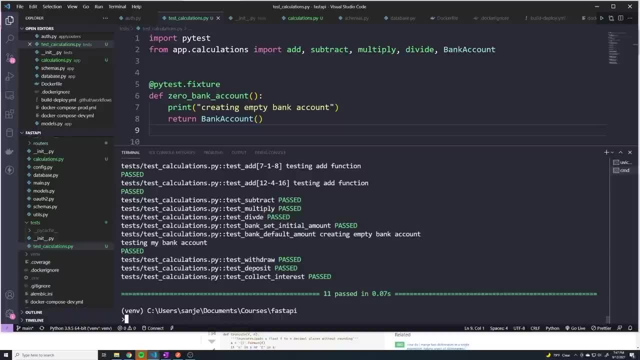 You can see that the code has been processed and I realize I have to pass in the dash s flag to see the print statements. All right, so here we go. We're going to test bank set initial amount. So I know test bank default amount, And so you'll see that when we start this test. 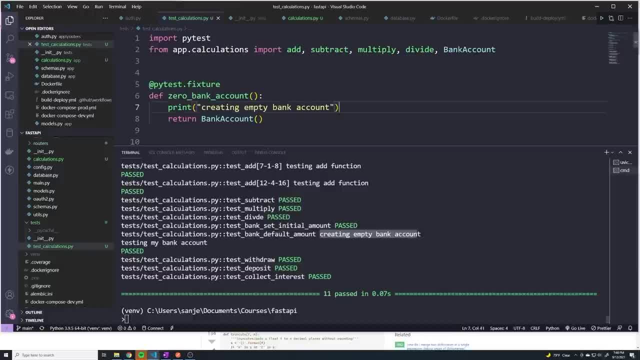 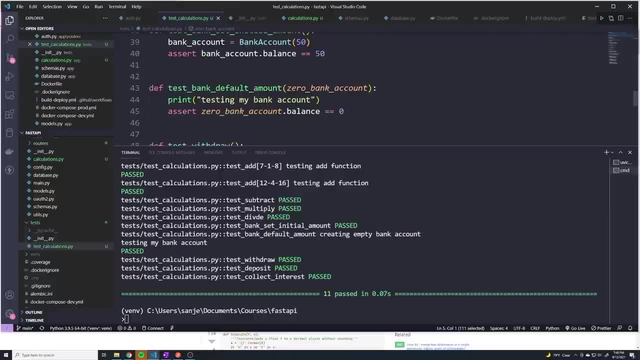 first things first is we create an empty bank account. That's that print statement for the fixture. So before the test even runs, we call the fixture because we've defined that here by saying: where is it that it's going to be a argument into the default amount test case. 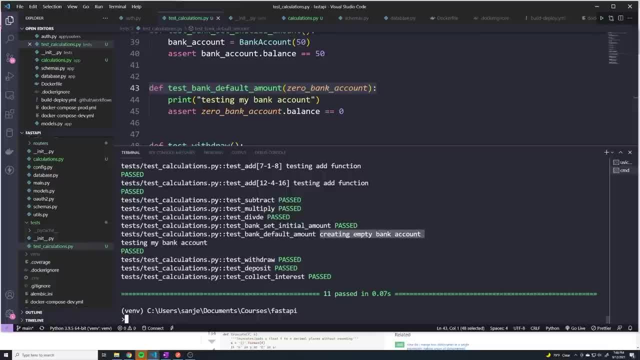 Then, after the fixtures run, which is just a function, we then run our actual test case And then we get the print testing my bank account right after that. So once again, just to really drive home this point: a fixture is just a function that runs before a specific. 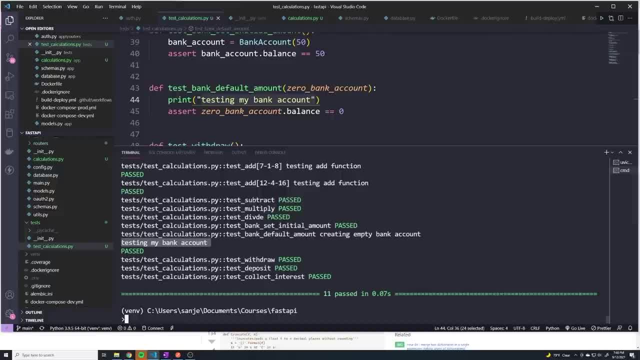 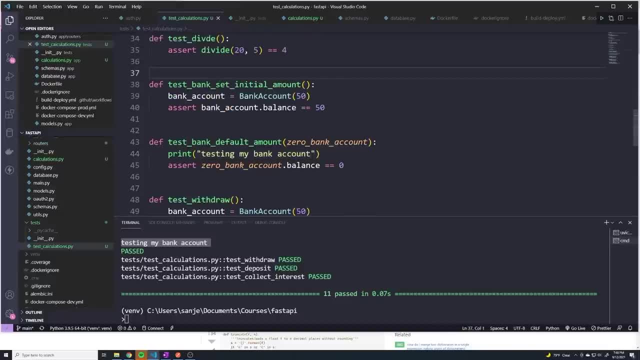 test case. That's all. But the great part is we can use the same fixture for all of our other tests. So let's go to the next one. So let's go to the next test, which is setting an initial amount, And in this case we have this. 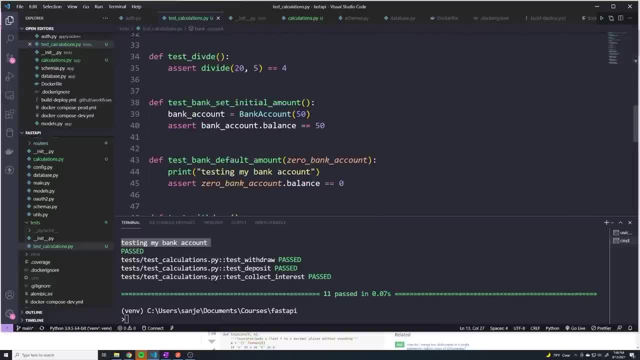 fixture right here, which is the bank account one, And so I'm going to say: this is going to go to bank account, So this will call the bank account fixture, and then we can remove this line And we can just keep this here, because it's referencing this variable now And this should. 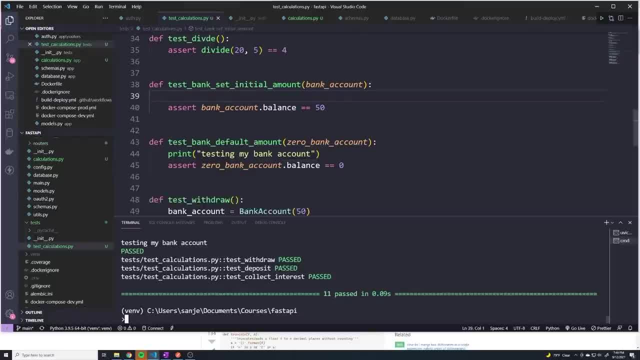 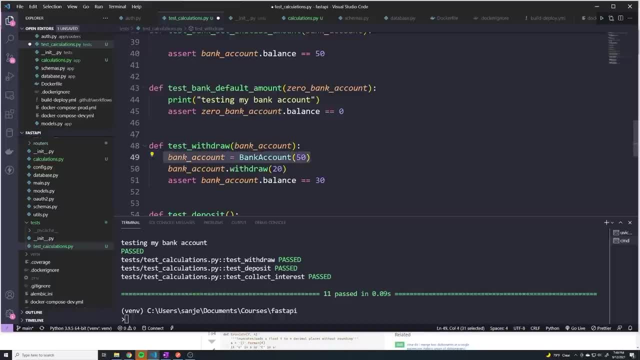 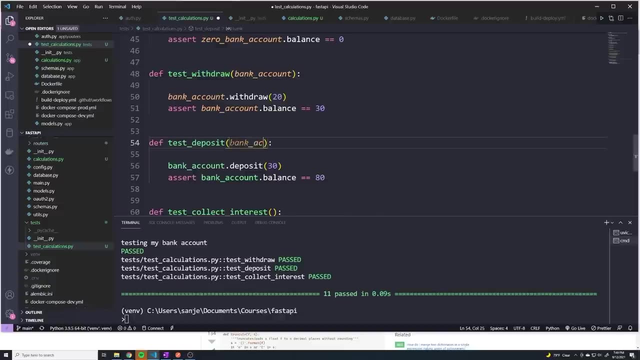 work now. So we run this once again. all tests pass And I can just do this for all of them. So I can just call the bank account fixture And I can just remove that line. Everything else can stay the same, and the same thing here as well. And finally, for the last one, we can do that, And so 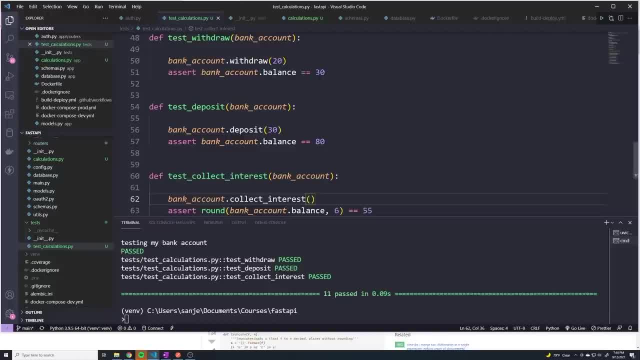 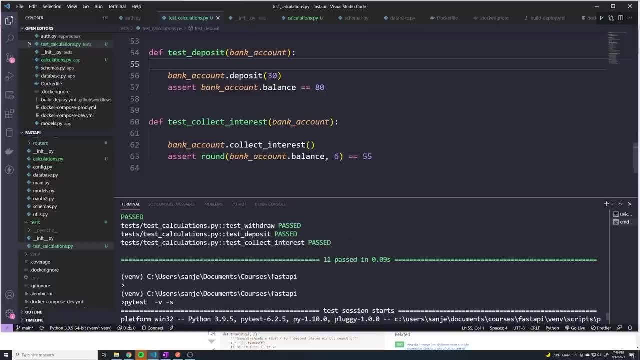 now you can see that we have saved us ourselves a couple of lines of code for each function, And if I run this, you can see that all the tests pass. So at this point you're probably thinking: you know, this doesn't really look like. 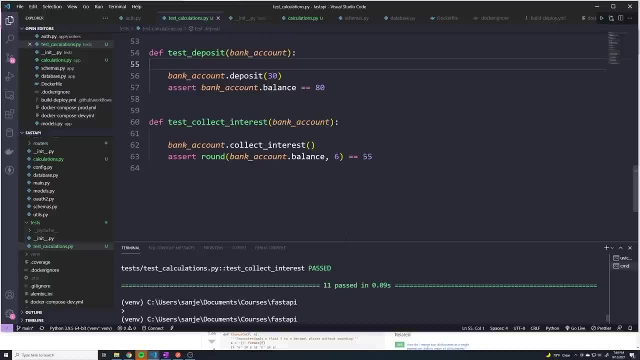 it saved us a lot of code, or a lot of you know coding out. However, there's going to be certain things that you want to do that you want to initialize before every single test of your entire application, So maybe something like setting up a test database, right? 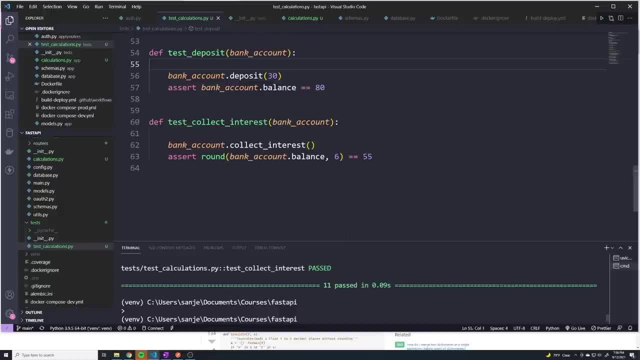 You'd want that to be set up for each single test. Having to manually do that for each test case would become very cumbersome, And then the lines of codes that you're repeating start to become a serious problem, And that's really one of the best use cases. 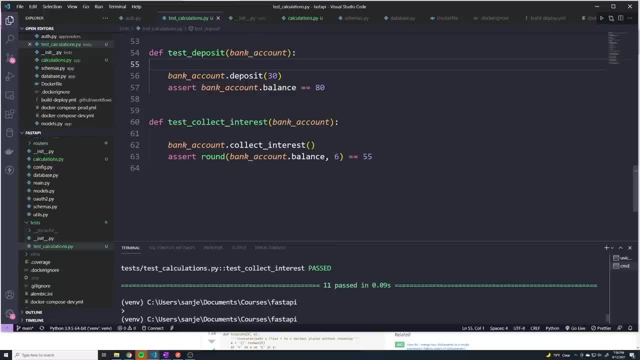 for using fixtures is something like setting up a database or setting up, you know, some sort of email service or something that you're going to use across a lot of your tests, And then having to initialize that manually for each test is going to be. 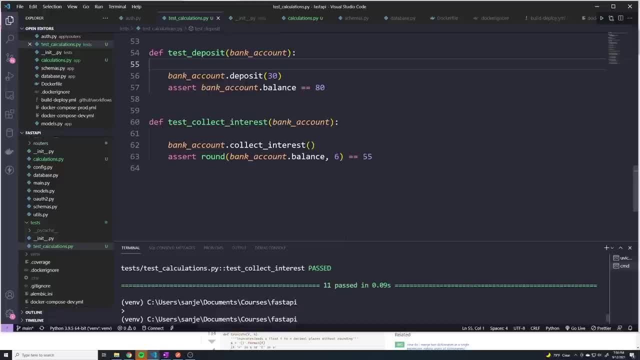 it's going to require a lot of work, And so that's where fixtures really help save us some time. Okay, what I want to do is I want to create one more test, And this test is going to be a little bit different. 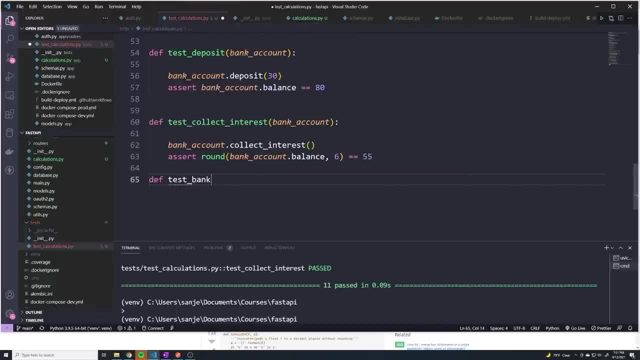 I'm going to call this a test about bank transaction maybe, And so this is going to test us both depositing money and withdrawing money in one test case, so that we can have a couple of different actions on a bank account. And so, just like we've done before, 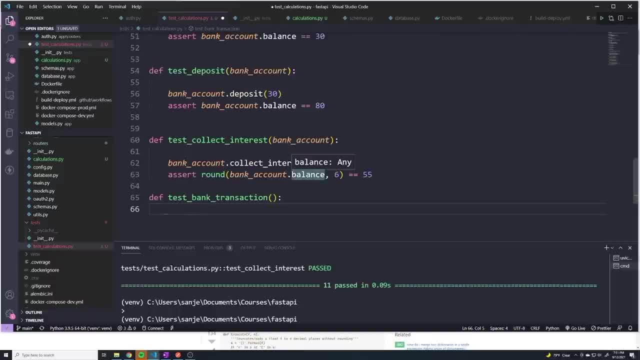 when it comes to, you know, setting up a fixture so that we can retrieve an instance of our bank account class, I'm going to do the same thing, but we're going to use the zero bank account, so it starts out with no money. 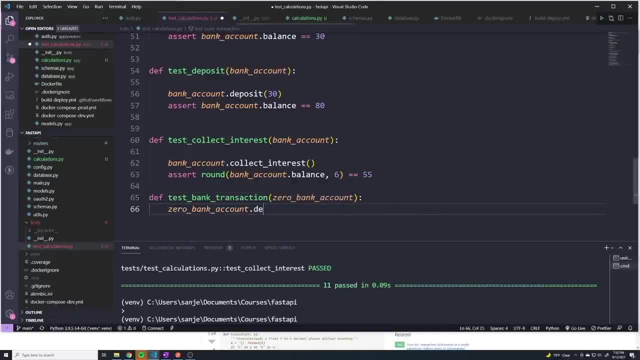 And then what we're going to do here is we're going to reference the zero and we're going to start off by depositing money, And let's say, I'll deposit $200.. And then we can also then withdraw an amount of money. 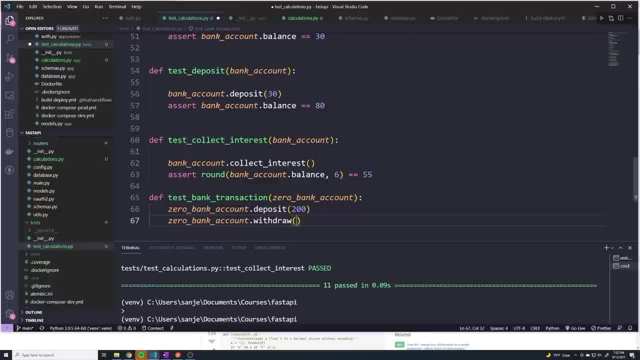 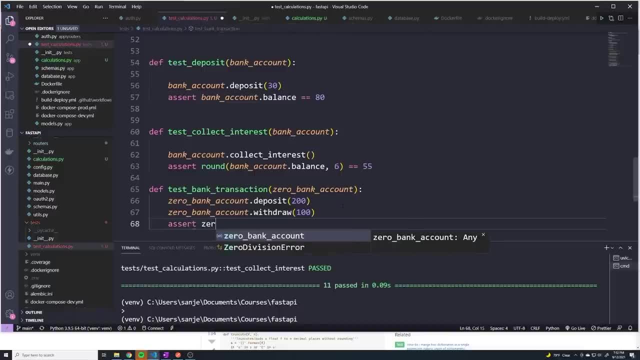 So now we're testing both in one specific test case And I'll say I'll withdraw $100. And we know that we should ultimately be left with $100. So we'll do: assert zero bank account dot balance equals equals 100.. So let's test this out. 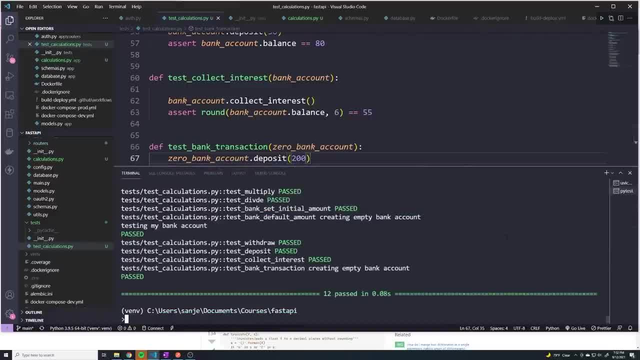 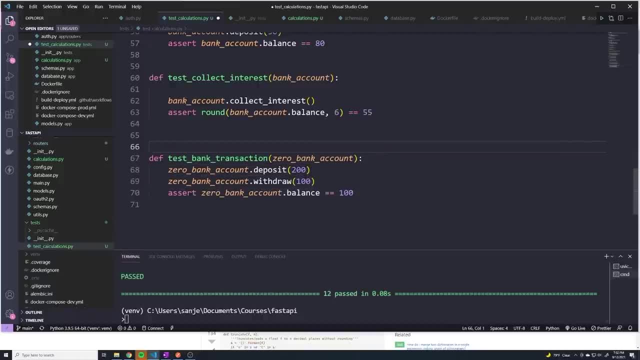 And let's see how this works. And that works as well. But what I wanted to do is for this specific test case. I wanted to show you that we can. we can use fixtures and parameterize so we can test multiple values, like we did for this specific test case. 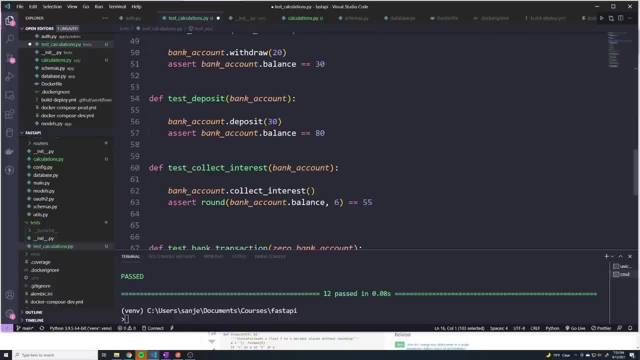 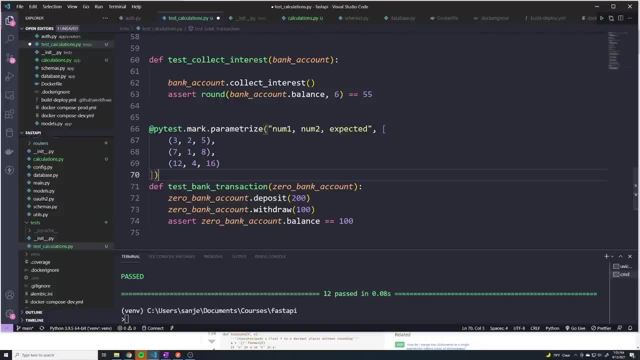 So what I'm going to do is I'm going to copy this so that we don't have to type this all from scratch, And we're going to create a couple of different test scenarios for this specific function, And in this case, we're going to have a deposited. 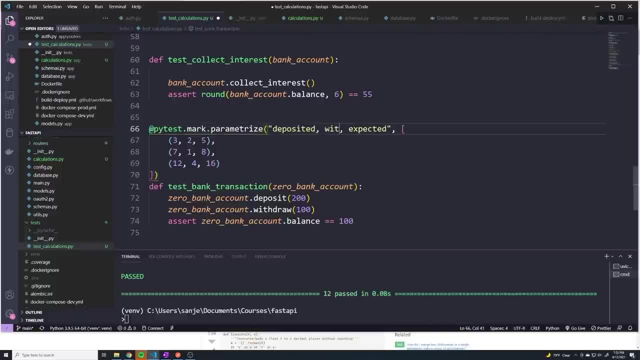 We're going to have a, we're going to have a withdrew, And we can have the expected amount And keep in mind you're not limited to having three variables. You can put as many as you want. It just happens to work out. 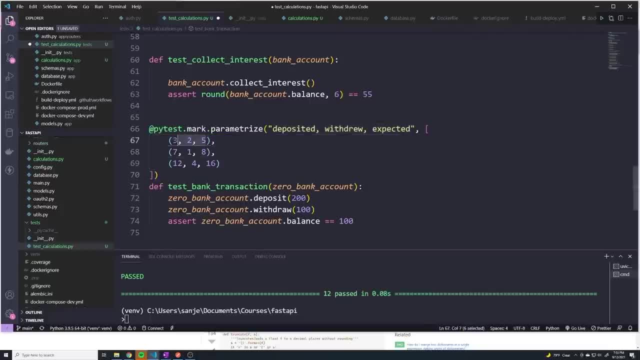 that I only need three in this case, And then we can provide some test data. So how about the same one we have right now? We're going to deposit $100, $200, sorry, withdraw $100. And we expect $100 in the end. 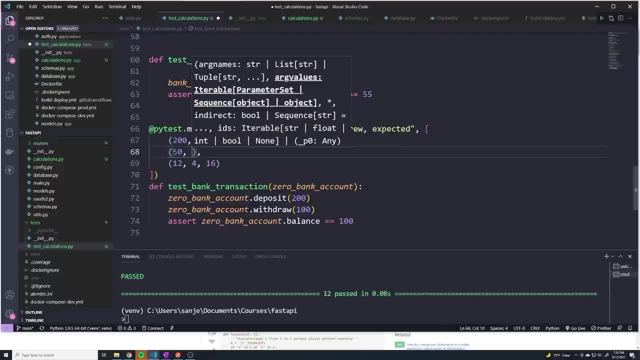 We can do the same thing. How about deposit $50,, withdraw $50, and we should end up with $40.. And then we've got our high roller, which is sitting there with a whopping $1,200.. And he withdrew. 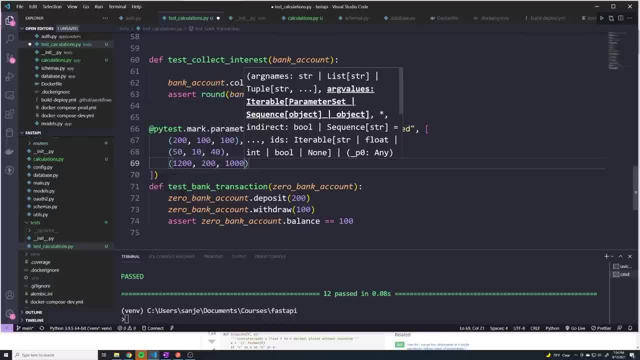 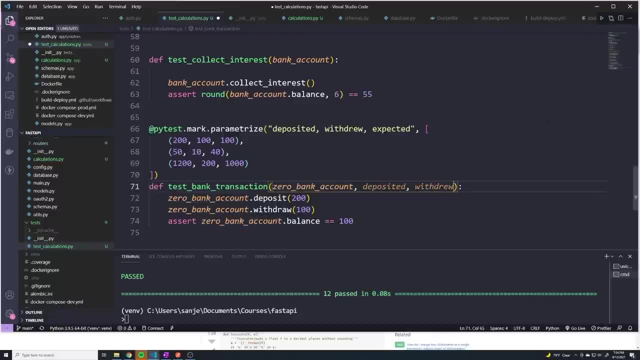 how about $200. And he's going to end up with $1,000 at the end. So now we can pass deposited, withdrew and expected, And now we can use deposited here, Withdrew here, And then we know what the expected is going to be. 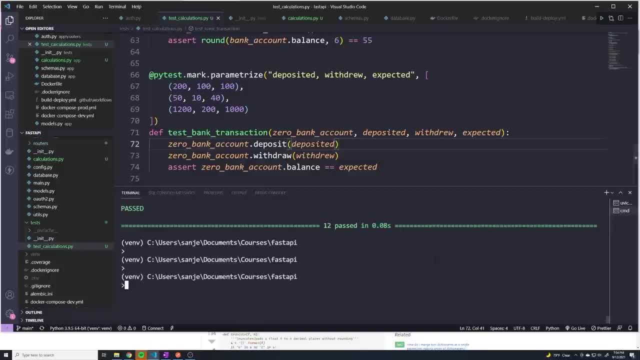 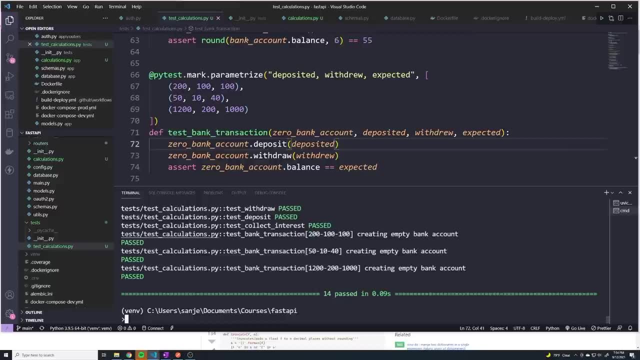 So let's try this out. All right, And we can see all three test cases run And, in this case, all three test cases passed. So I just wanted to show you guys that you can use this with our fixture. So it's okay if you're using a fixture. 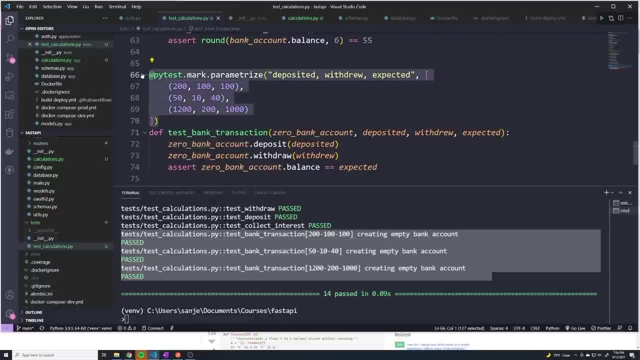 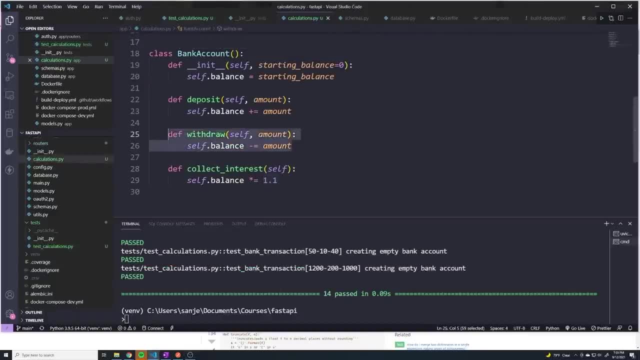 you can still use the parameterize decorator in this case to test multiple scenarios. If we go back to our bank account class and you take a look at the withdraw method, you'll notice that right now we're not performing any check to make sure that the user. 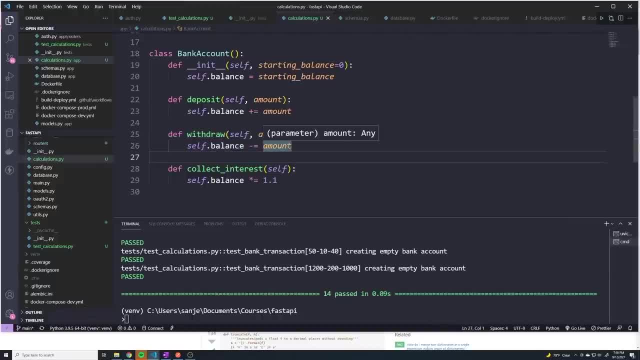 has enough money. And that's not really how a bank account works, because if you have $100 and you withdraw $500, the bank's going to be like we can't do that. So it just makes sense in our code to actually perform. 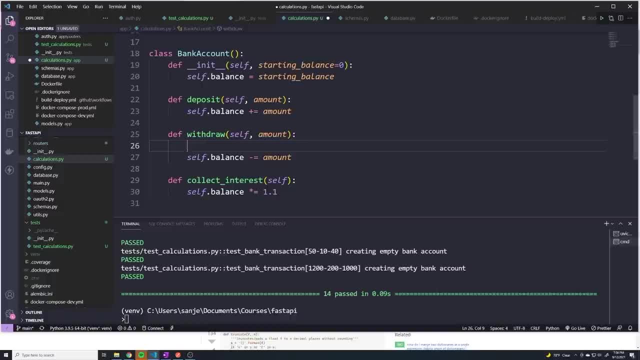 some sort of check, And so usually you know something simple is we'll say, hey, if amount that you're trying to withdraw is greater than your balance. well, what are we going to do? Well, we're probably going to raise an exception. 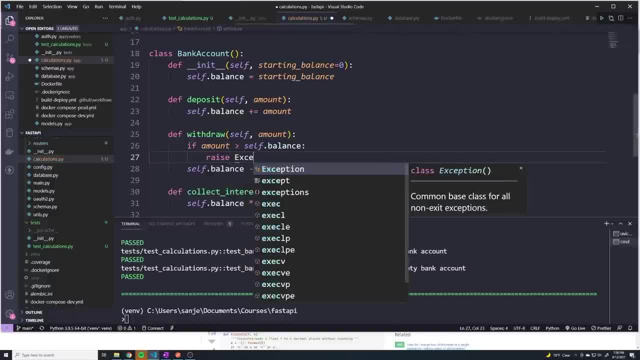 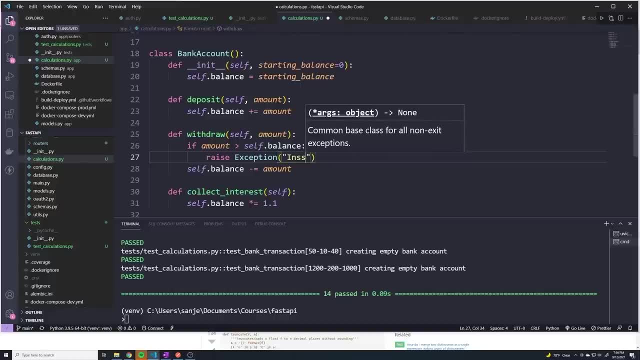 So I'll say raise, and we're just going to raise a standard Python exception. and we'll just say something: hey, insufficient funds in account, Right. However, if we do have enough money, then we will actually perform that operation. So this is all good. 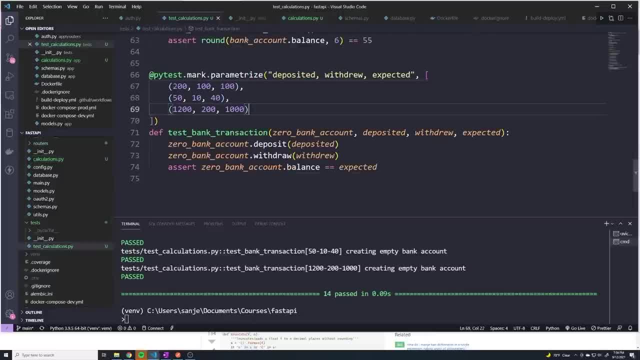 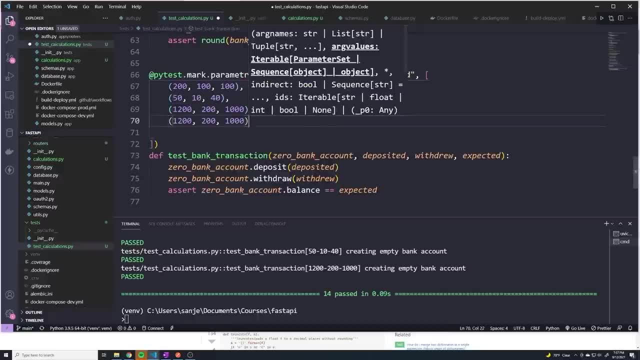 If we go to our test calculations and we just add one more scenario in this case, But this time we deposit, let's say, only $10, and we try to withdraw I don't know 50. Well, what is the expected scenario? 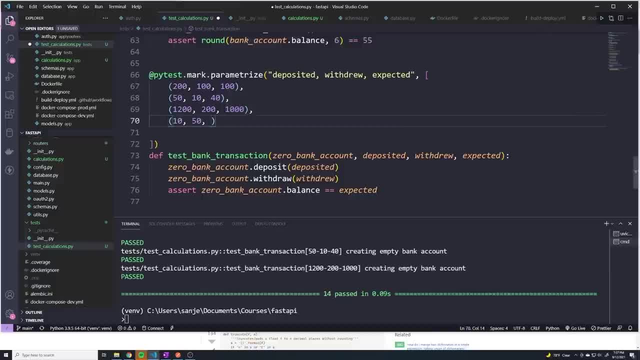 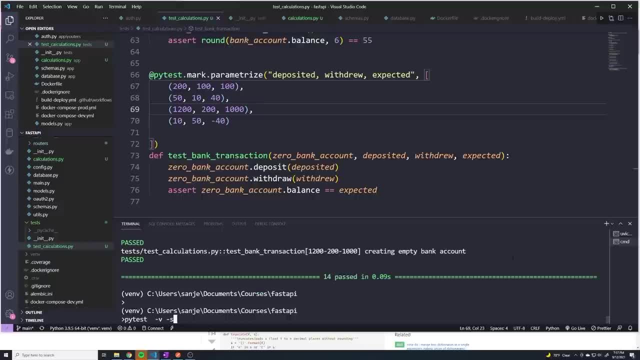 The expected value, And it doesn't really matter what we put in, because this is ultimately going to, you know, break, Break our code because we're raising an exception. So if I try to run this Right, it's going to fail. 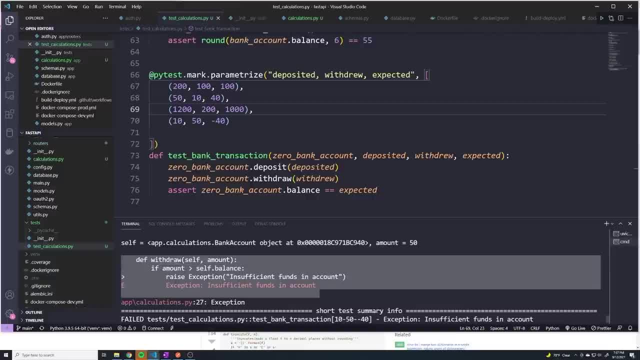 Because we're raising an exception And remember, anytime you throw an error, that's going to automatically make the test fail. So what do we do? Well, first of all, let's remove this test case, because for scenarios like this, where you expect to receive an error, 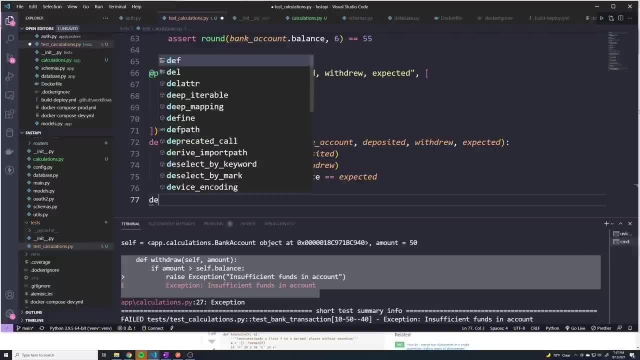 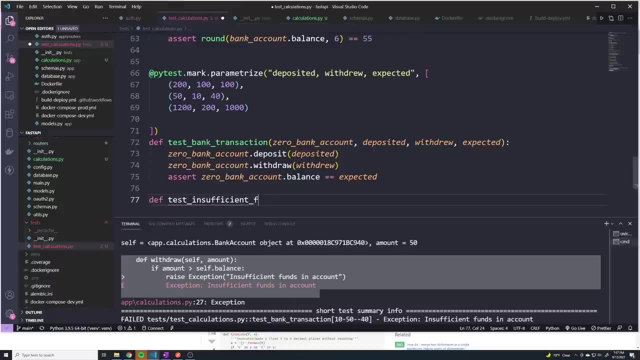 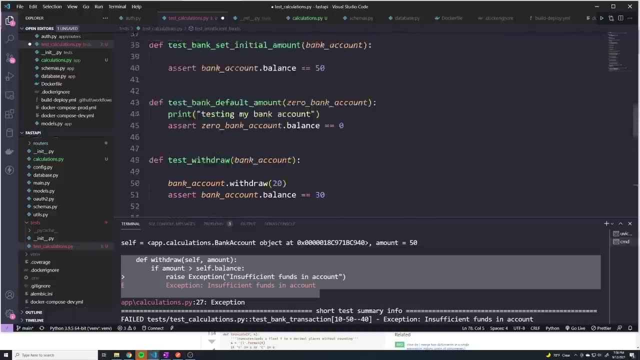 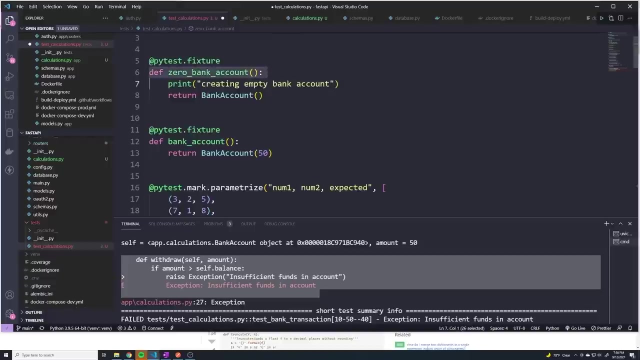 we need to create a different test case, So I'll call this: Well, how about test insufficient funds? And let's say we start out with, instead of using the zero bank account, where is the? instead, instead of using this bank account, we're going to use the zero bank account. 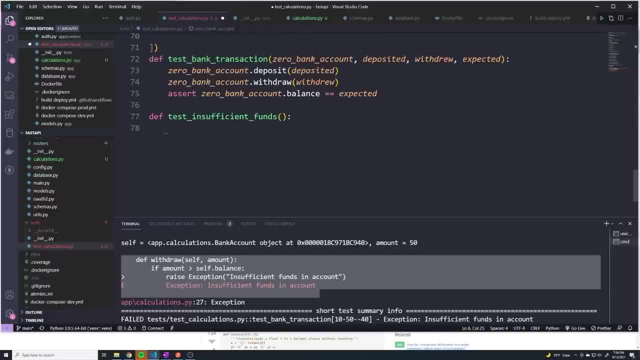 and then we'll just try to withdraw money. So that's an easy way of testing it. So we'll say zero Underscore bank account, So we'll have no money in our account And we're going to withdraw some money. 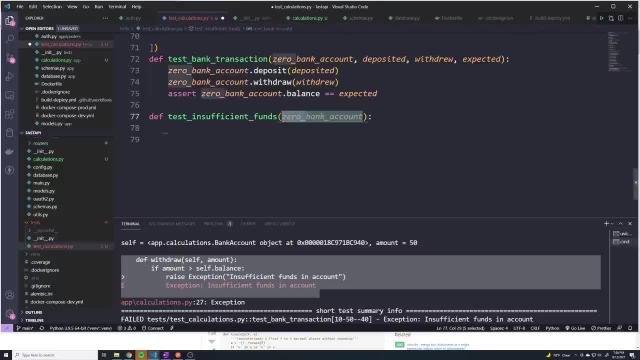 So we would do. you know, actually I'll just do a regular bank account. I don't know why I want zero. So we'll start out with Fifty bucks and we'll try to do a bank account. Dot withdraw And we'll try to withdraw two hundred dollars. 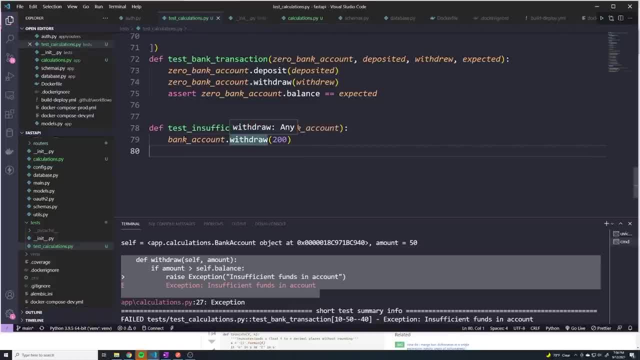 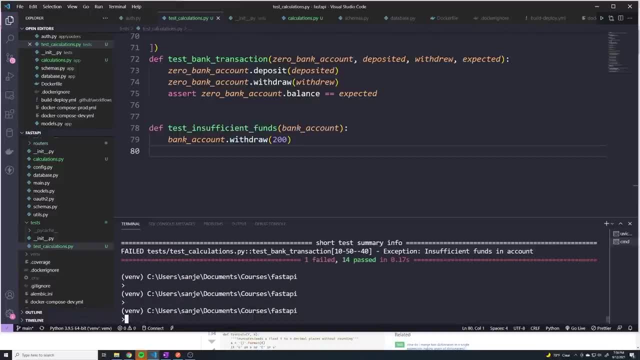 So that should raise the exception. But how exactly in our test do we tell Python it's expected to receive an exception? Because right now, if we run this once again, we're going to get the same exact error: Right Failed. So what do we do? 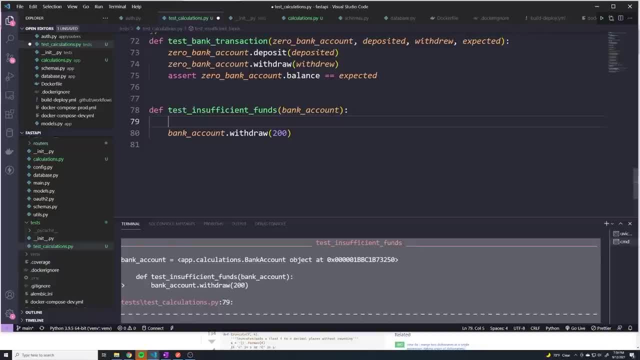 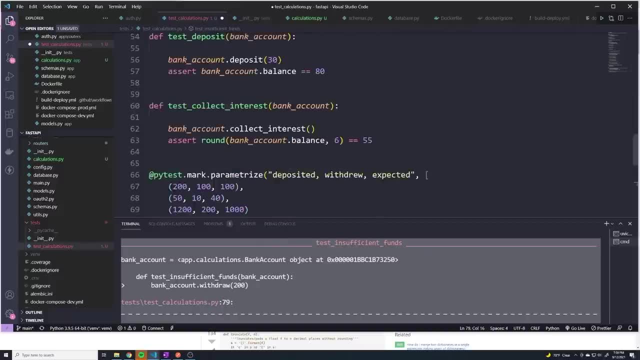 This is how you tell Python that you accept, that you expect an exception you do with, And then you call pi test. Remember we imported pi test all the way at the top, Right here, So we'll do pi test. Dot raises. 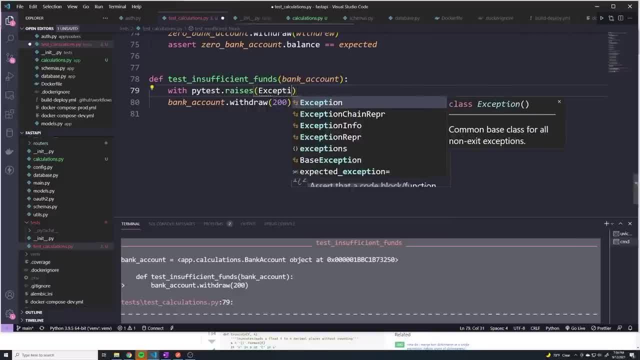 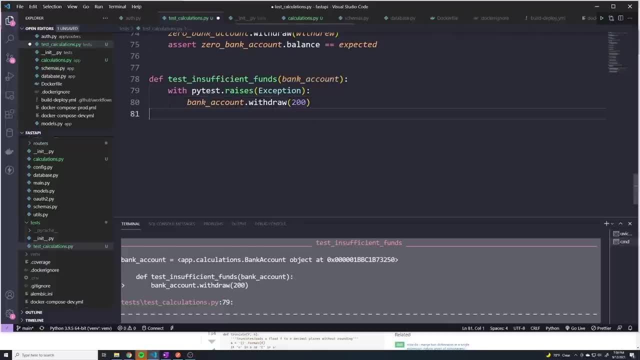 And then you provide the exception that you expect. So in this case, this is just a regular Python exception, So you can just say that, and then you provide the command that you're going to run. OK, and so that way, if this command throws an error or 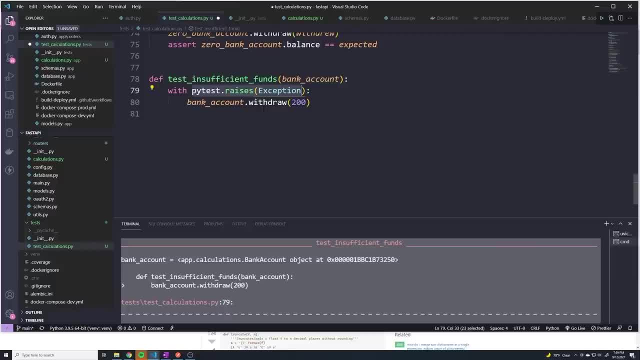 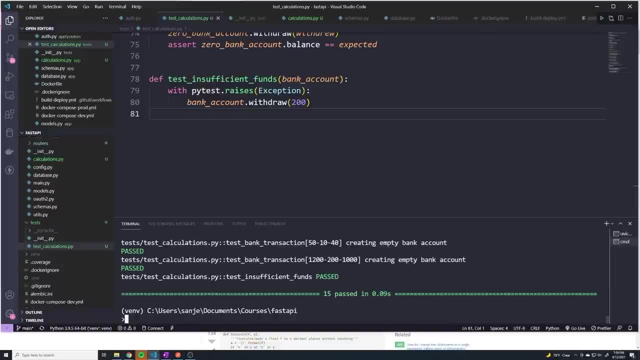 raises an exception, pi test will be told to expect this, so then it would consider the test as passing. And now if I run this, We can see that the insufficient funds test passed. And if we go back to our code and actually remove this exception, 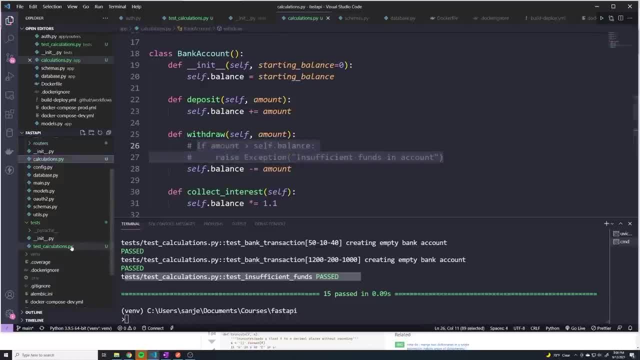 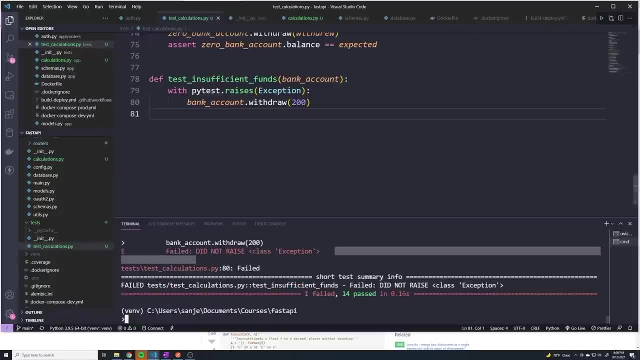 We'll comment out that entire statement. What do you think is going to happen here Right now? it's failed because it did not raise an exception. Pi test is expecting an exception and we didn't raise one, So then it considers that a error in our code. 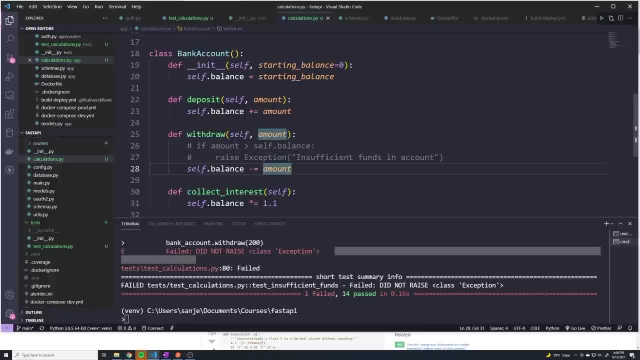 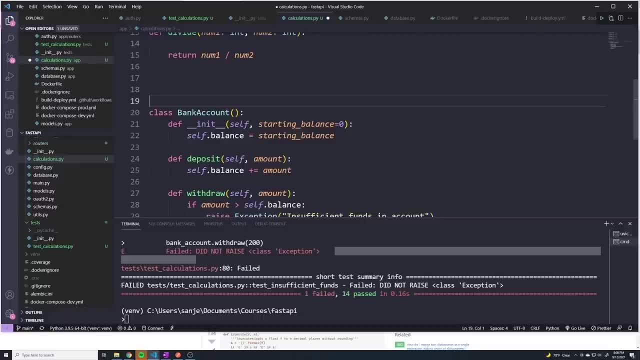 because when we expect an exception, we should expect an exception. So I'll uncomment this. And now you know in real code, right, you wouldn't just throw just a generic Python exception. you're going to usually create your own exception classes. 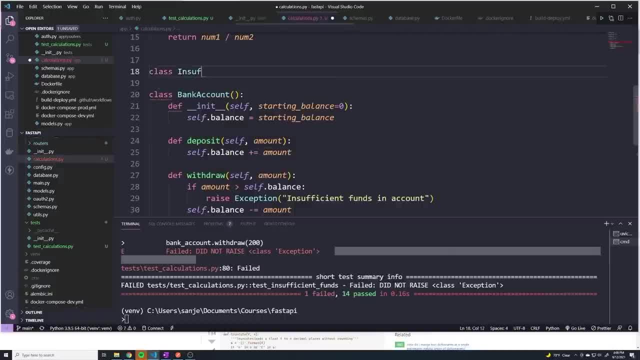 So let's say we define our own exception and I'll call this insufficient Funds, and this is going to extend the exception class And we'll just say there's no property, so I'll just say pass. And in this case I'll say we'll raise an insufficient fund. 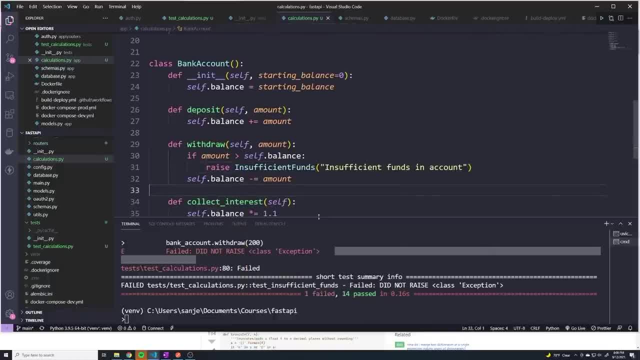 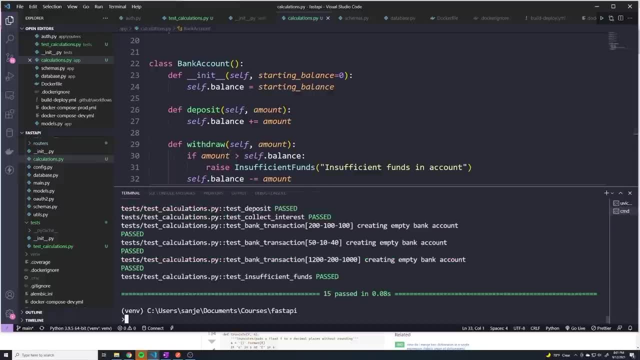 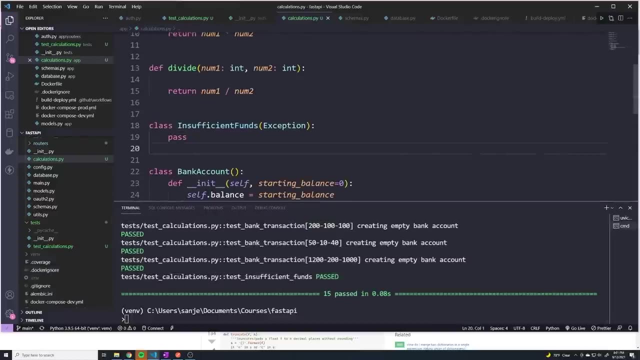 Insufficient funds. All right, so if I make this change, What do you think is going to happen? You think it's going to break our code. Well, let's run this. We can see that it passed, And the reason why it passed is because insufficient funds is a child class to the exception class. 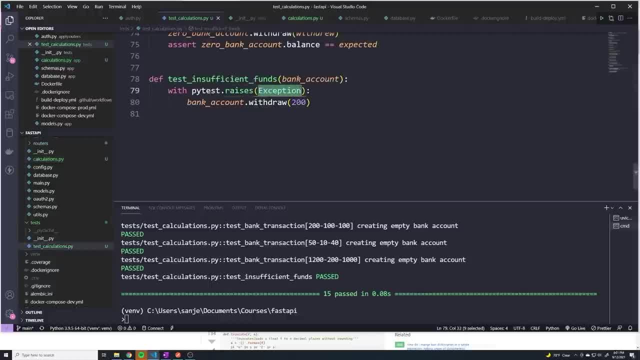 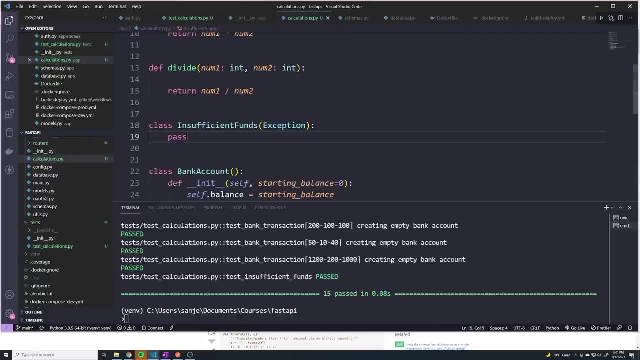 So when we say we accept, we expect an exception, technically we are getting the exception. It's just we haven't specified we specifically want a insufficient funds Exception. and because this is inheriting from this class, Python says: Hey look, everything looks good. 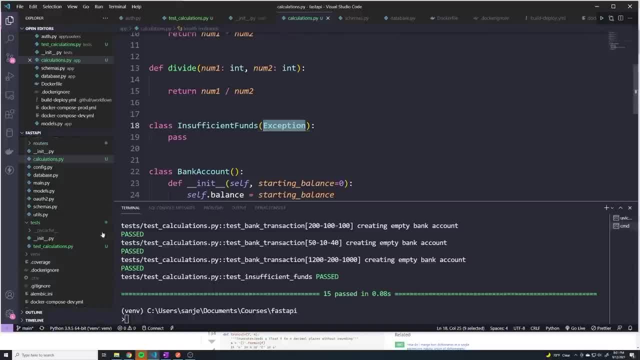 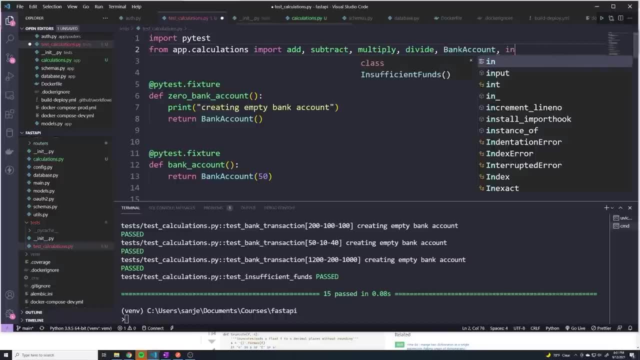 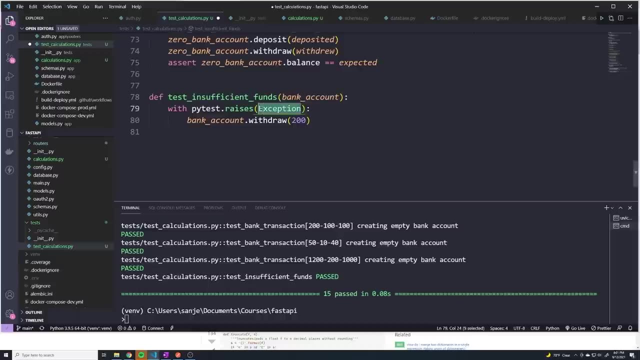 But if you did want to be as specific as possible, which is generally recommended, what we can do is: I can import that exception. So we'll say: from app dot calculations we can import insufficient funds. And now here we can say: we expect, we expect a insufficient funds. 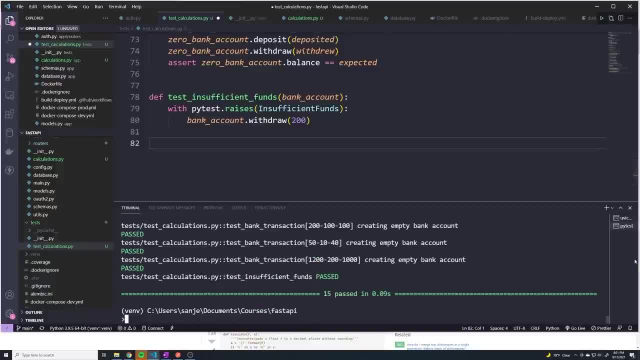 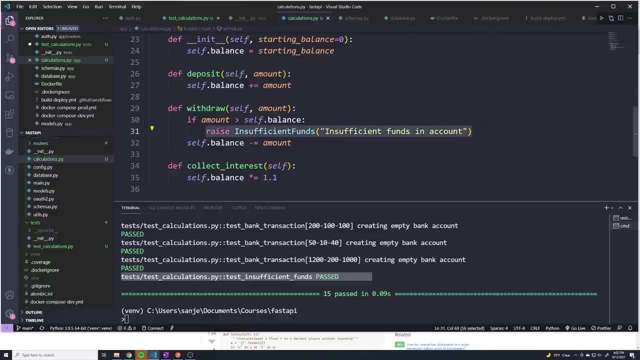 And so now, if I run this, we can see that it passes. And the benefit of this is that if, for some reason, our code raised a another type of exception, it would consider this test as failing. So if I go back to my code and let's say that, you know, for some reason something broken our code and all of a sudden, instead of raising an insufficient funds error, we get some other kind of exception, 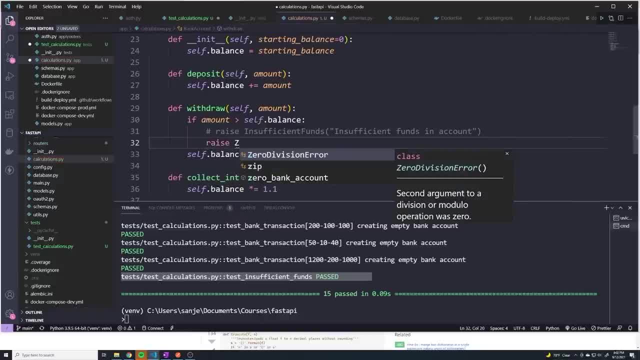 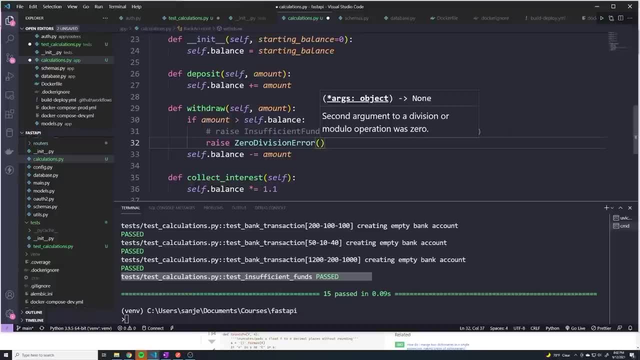 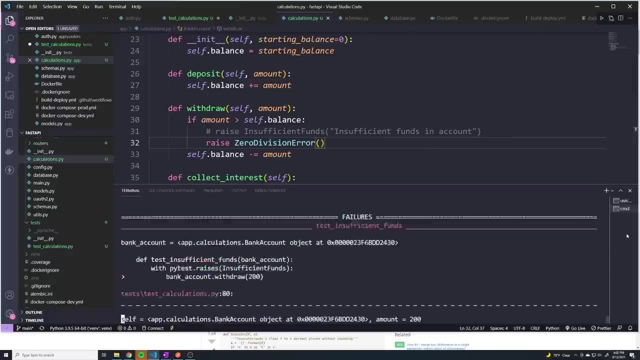 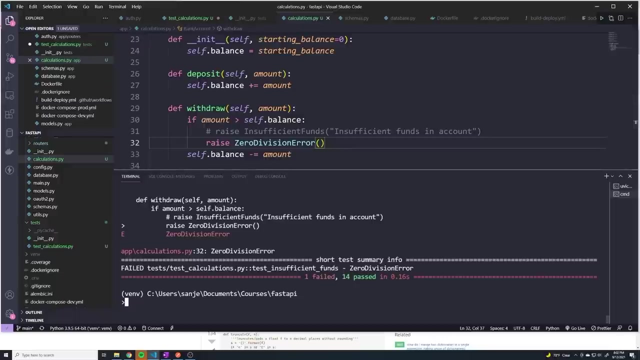 And I can just simulate this by doing raise Zero division error. So if you ever try to divide a number by zero, this is the the exception that's expected. And so now, if I run this right, we can see that the test failed because we expected a insufficient funds exception, but we got a zero division error. 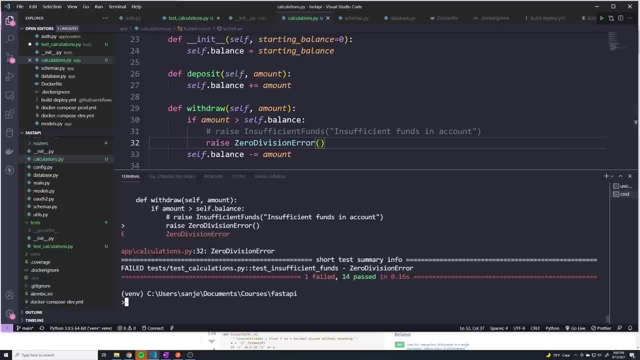 And so that considers the test as failing, because we've told that we've expected Something but we got something else. So it's generally best to explicitly define the exact exception that you expect, so that you can make sure that you know that nothing else is broken, because technically any part of your code can break and throw an error. 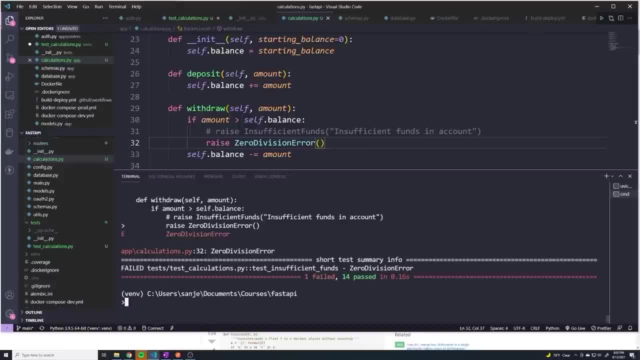 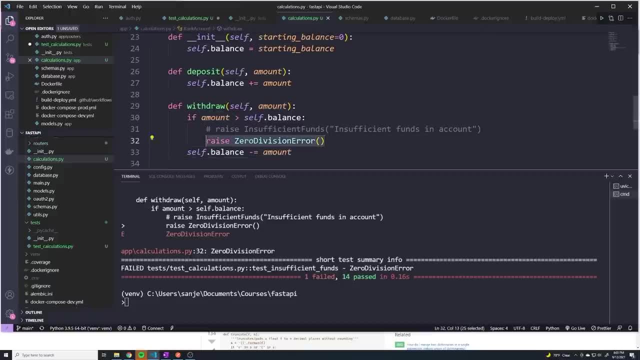 And if it throws an error and we just try to, if we just tell you know our test to expect any exception, then it may not be doing what we actually expect it to do, But we'll change this back. We don't need that anymore. 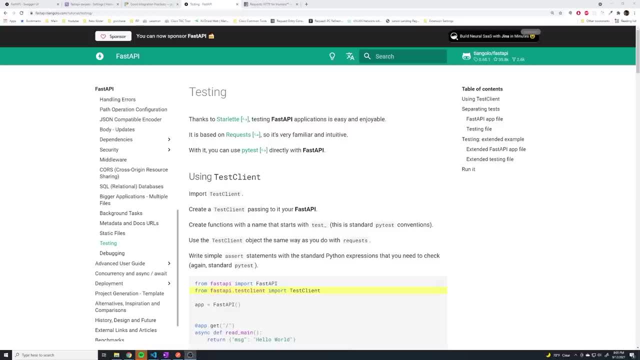 Okay, so I think we have a good enough understanding on how to create Create a test, And I think it's time we actually started testing our application When it comes to fast API. fast API automatically provides us a test client, So all we have to do is we just say: from fast API, dot test client, import test client. 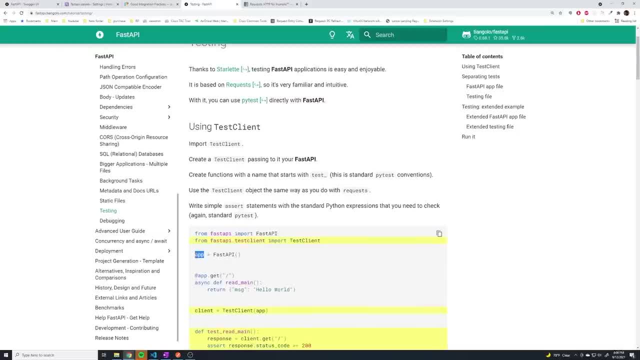 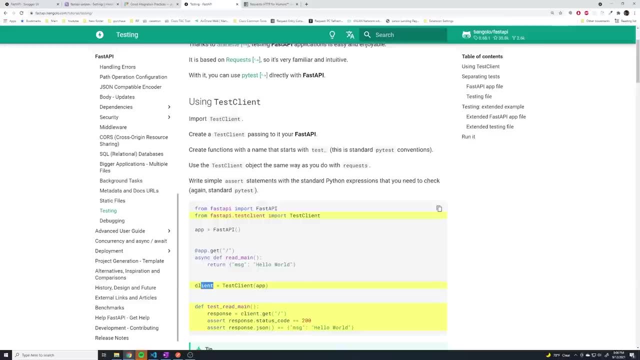 And then all we have to do is then just pass in our fast API instance, which is stored under the variable app, And then we can just perform any requests to our application by doing client, which is what we named the test client, and then just doing a dot get or a dot post or whatever. 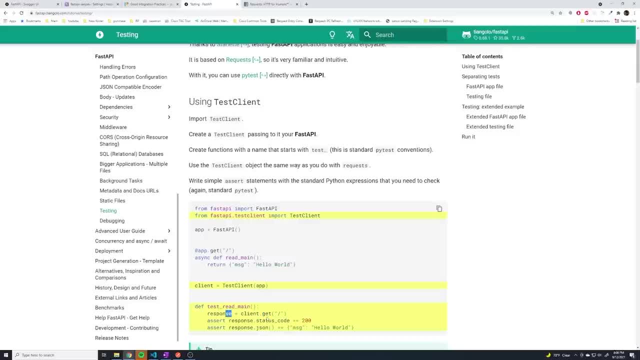 And then we can get the response, and then we can assert anything that we want, just to make sure that we get the responses that we ultimately expect And keep in mind when you make use of this test client. if you take a look at the documentation, it says that you use this the same way you would any requests. object: 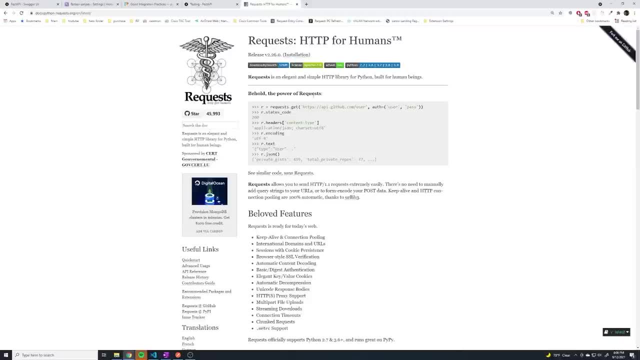 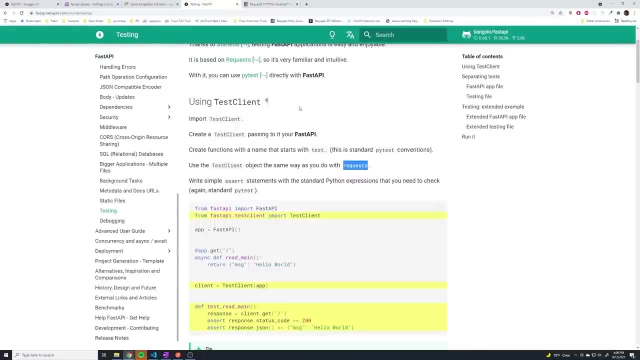 So if you've ever used the request library from Python, this is the same exact object. So anything you could do with requests you can do with the test client so you can customize the request, you can change the HTTP method, You can add a request. 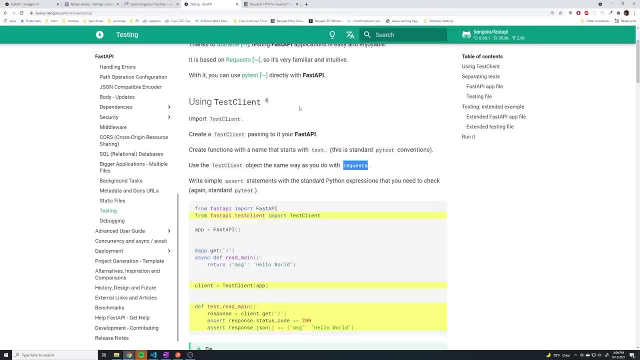 You can add a body, a payload, You can add a authorization header. It's really just doing what Postman is doing for us, but we're going to do it through code instead of manually opening up Postman and then you know, figuring out which requests we want to send. 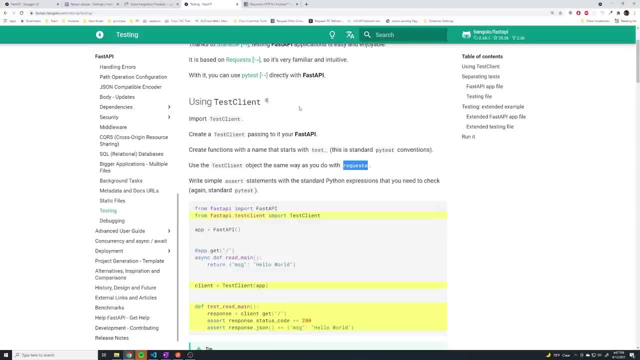 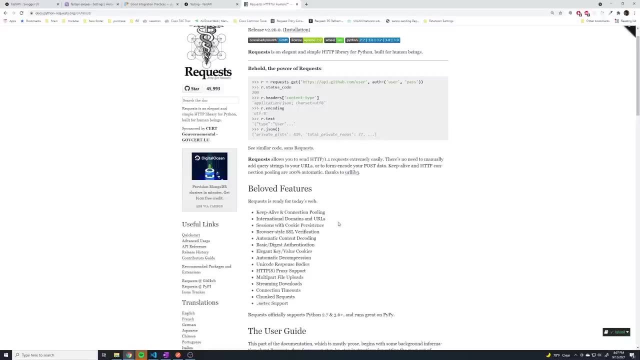 We're just going to do it out in Python so we can do it all in an automated, automated fashion. But if you haven't worked with the request library, definitely take a look at this. Just take a look at how we generate requests. It's not too difficult, right. 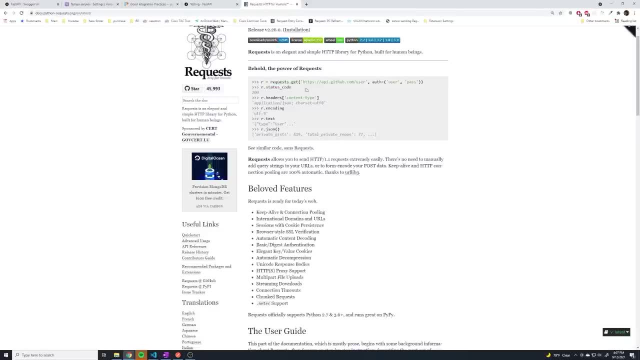 It's just request dot get or in our case we're going to call a client, but it doesn't really matter- And then you provide the URL that you want to run This against and then you know you can add in other properties like an auth header or anything like that. 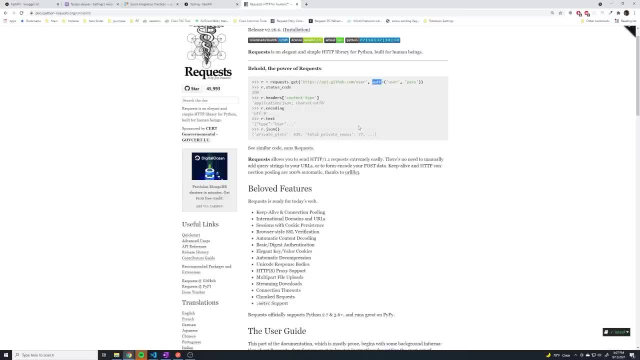 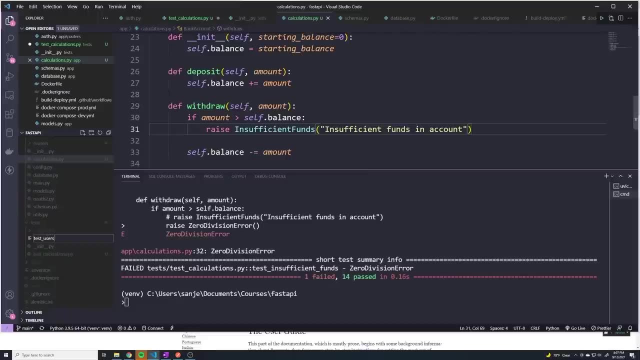 So it's just about customizing your specific HTTP request, And so I'm going to create a new file and I'm going to call this: How about test underscore users? This, this module, represent tests for, you know, creating users and and getting users profiles, information and things like that. 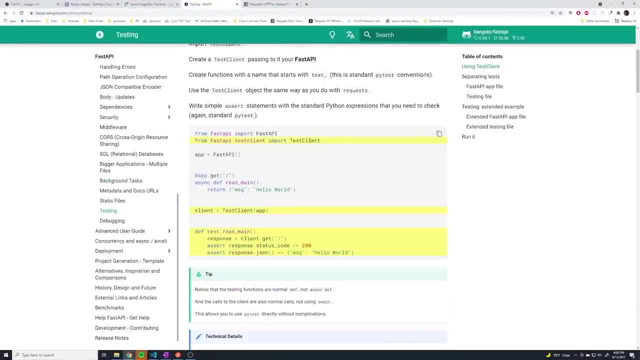 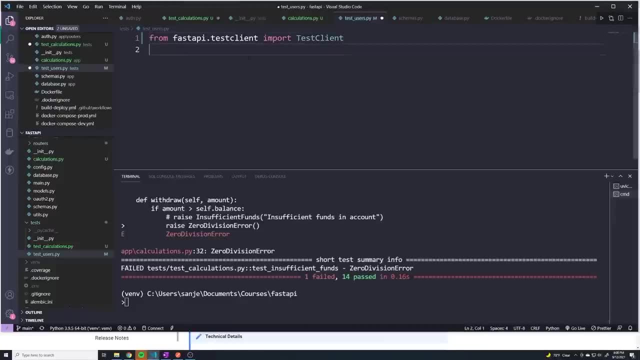 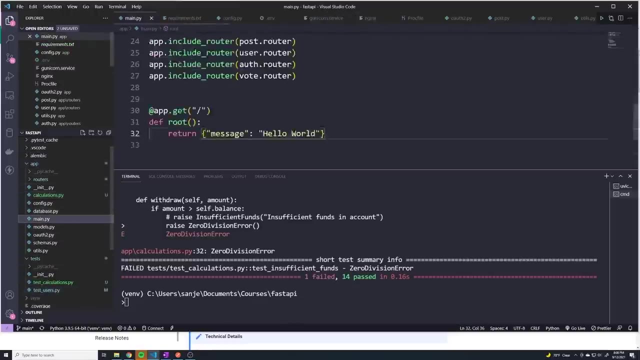 And just like it shows in the file Fast API documentation, Let's just copy this line right here And then what we want to do is: we want to import from our app package, go to our main file. We want to import our our fast API instance. 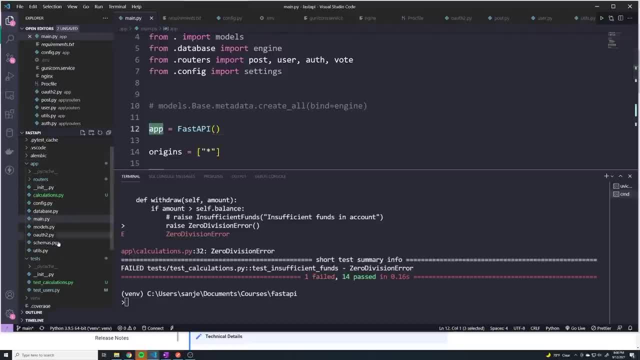 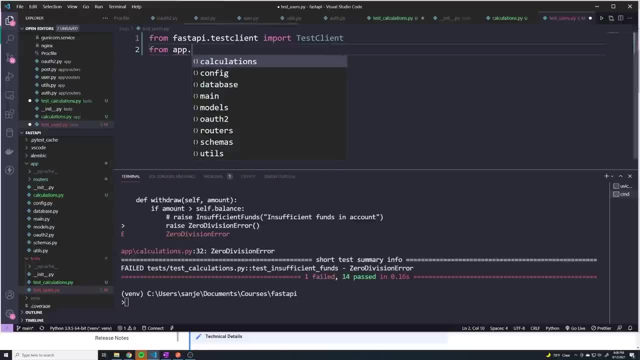 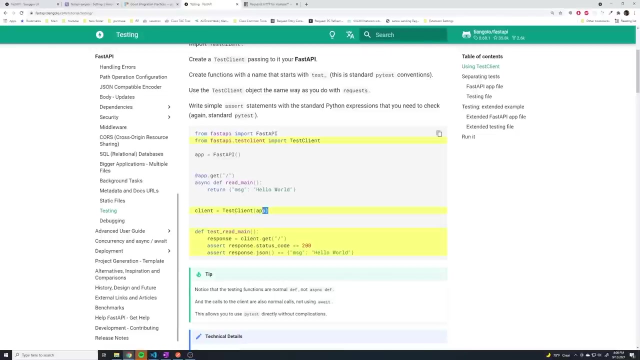 So we want to import this app right here, so that we can actually test it. I'll say: from App dot Main, Import App Right. so we have our app instance And we'll just copy this line right here, which is just: 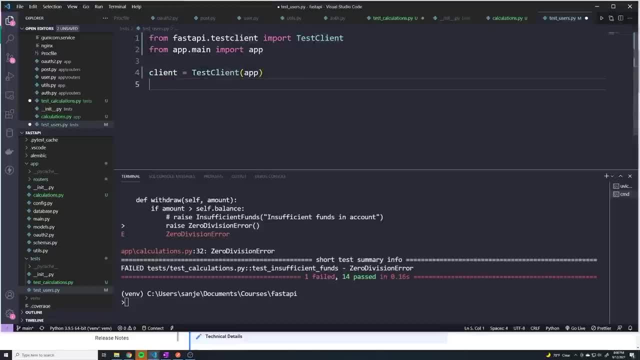 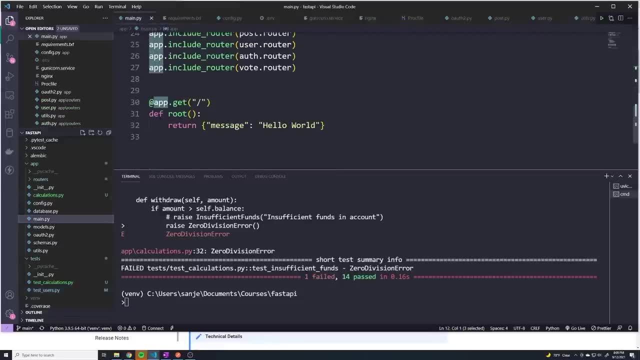 Setting our test client To a variable called client, and so now we can run whatever tests that we want, And I think you know. just to keep things simple, let's start off with the simple route path that we have right here. 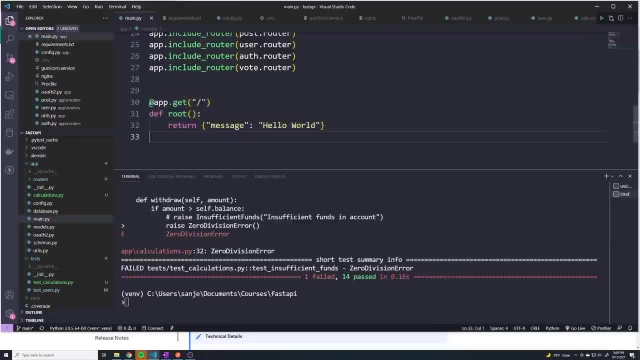 Just a test that this works, Because that way we don't have to worry about authentication or error passing any other data. Let's start off with the simplest scenarios. So this is at the root URL. So we will go to our test users. 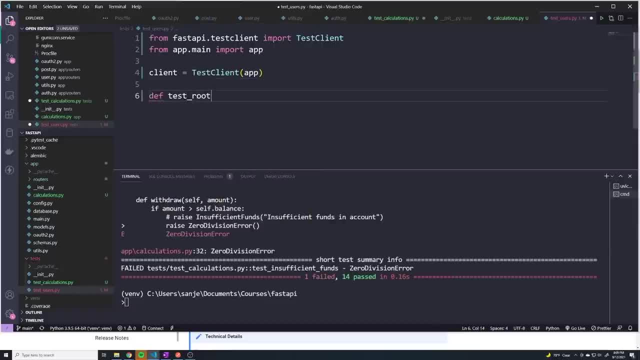 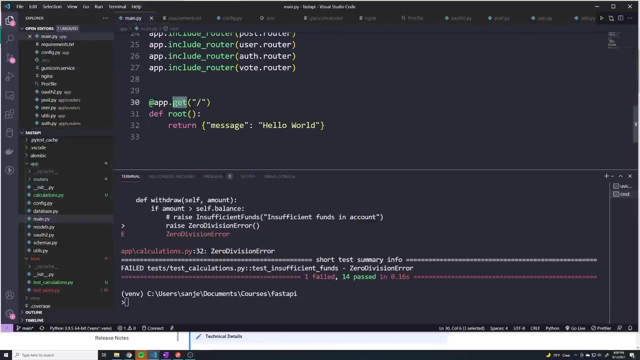 And I'm just going to call this test route Because it's not really a real function or anything like that. And then here we'll say: client dot, And since we are testing a specific path Operation, this is a get method. So we want to send a get. 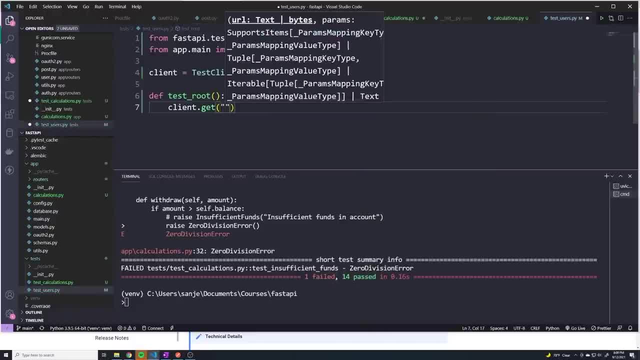 So we'll do client dot. get Then the URL, So we can just say slash. We don't have to do you know local host, because it's not technically a running server. We actually just pass the actual app instance, So we just say the route path. 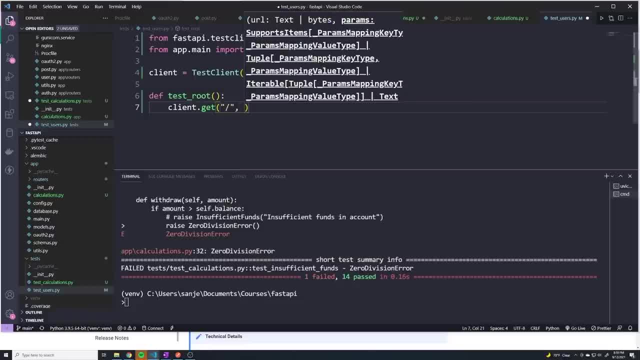 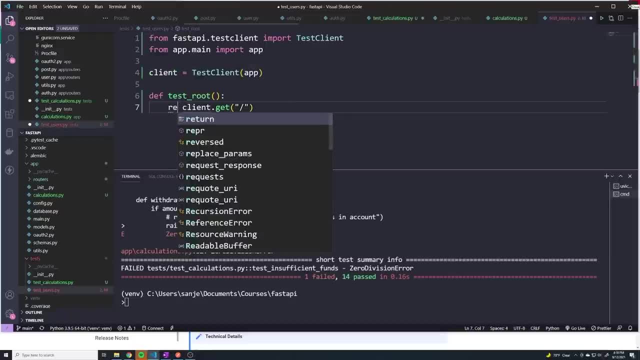 And then you can pass in other things like you know what, payload and things like that. But we'll leave that for now. Now leave it empty and we'll. we'll store the response Under a variable called res And instead of doing an assert or anything like that, for now I just want to print out: 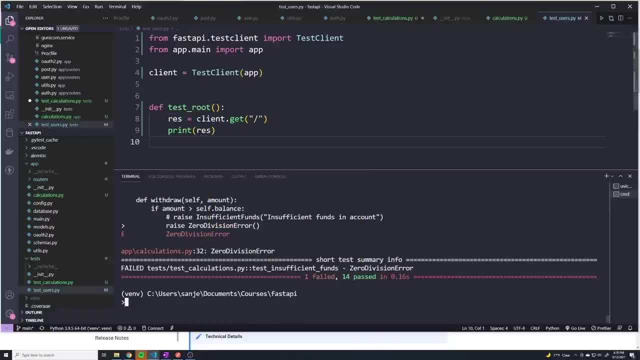 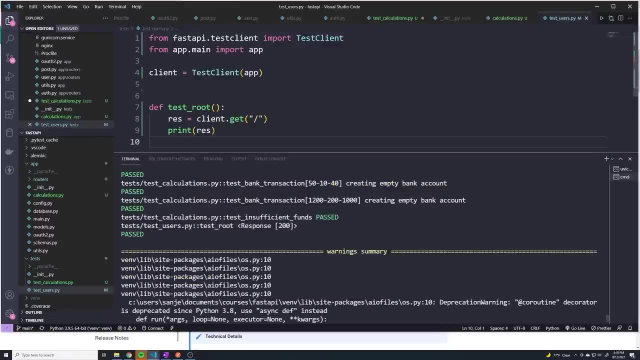 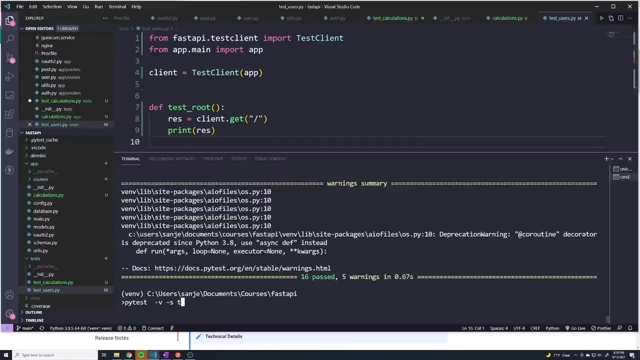 The response: All right, and if I run this, Okay. so a little bit annoying thing right now. it's going to run all of our tests And if you just want to test one test or one module, then I recommend you just do the same thing, except pass in the path to just your specific. 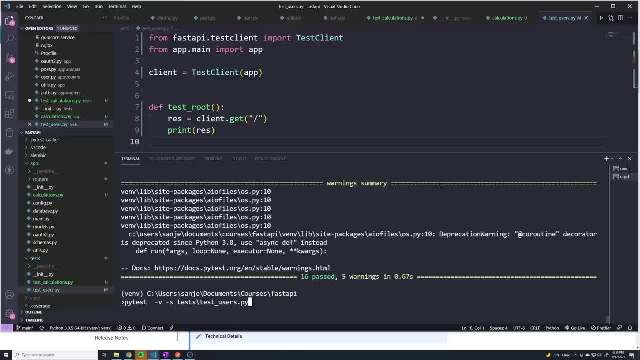 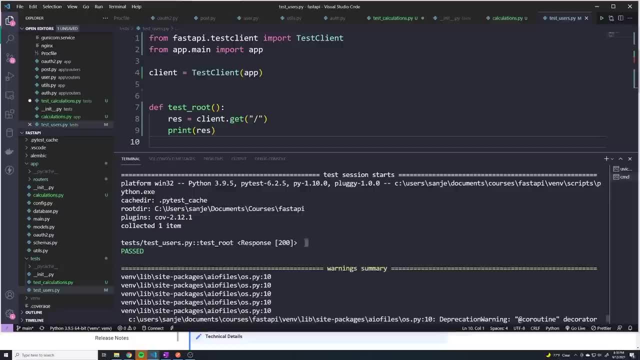 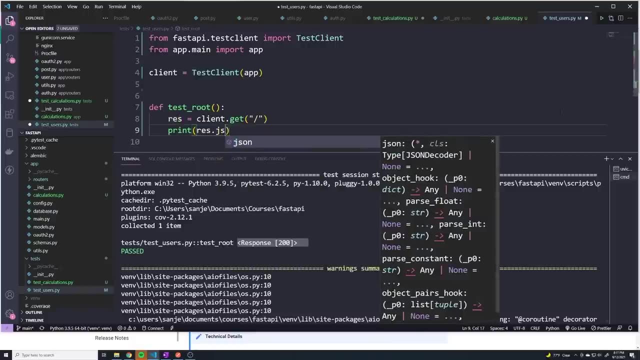 Your specific module so that we don't run all of our tests all over again. so we can just run one in this case. And if we take a look at this, We can see that it just prints out a response object, not very helpful, but if you want to see what's the actual payload, we can say dot, chase on. 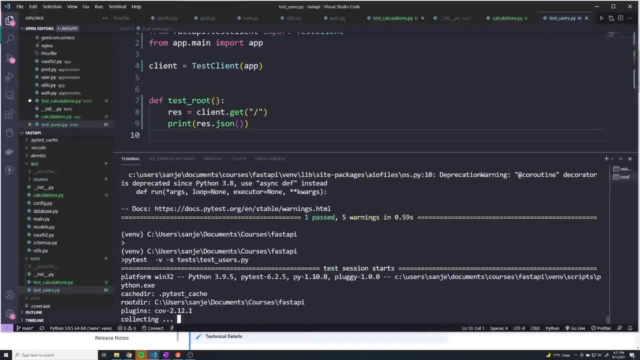 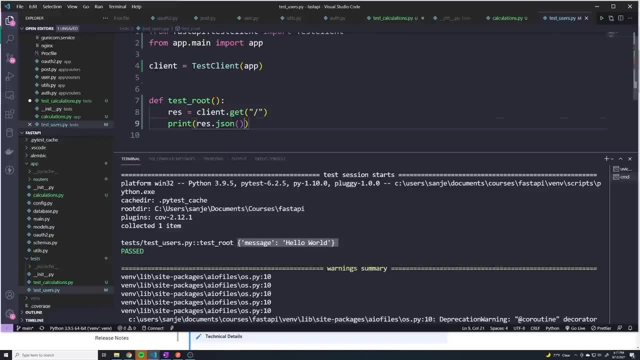 To see what the data looks like, And so then I can run this And we could see that, hey look, we get message Hello world. And if I Wanted to grab The message property I could say: dot get. 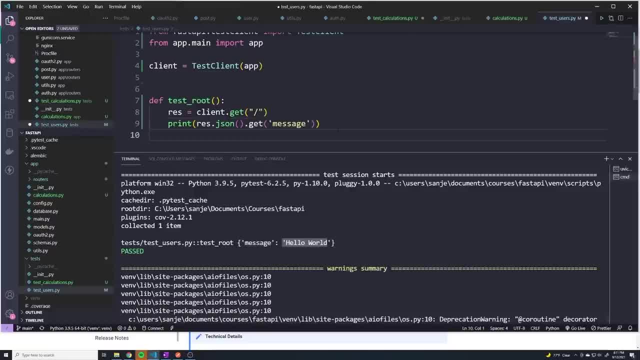 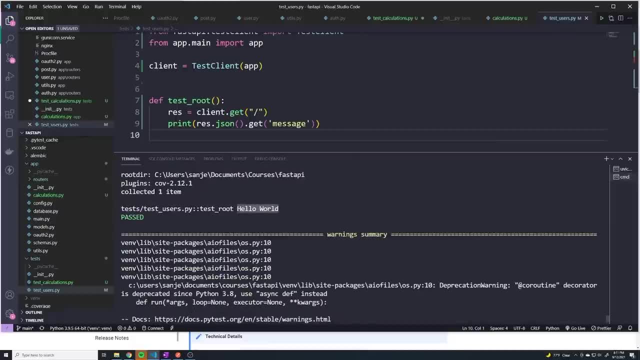 And then message and it should return: Hello world. Let's try this out one more time And we could see that it prints out Hello world. So to test that this route actually works, what we can do is we can just do an assert. 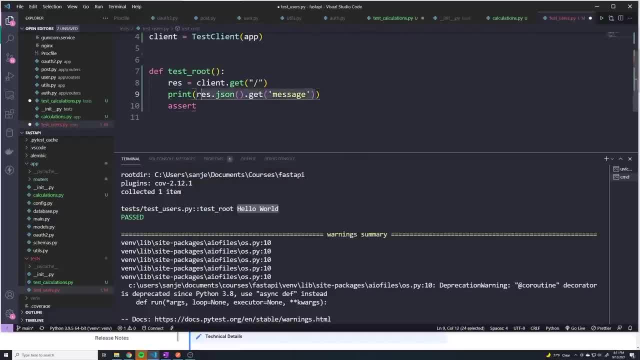 And I could say assert. and then literally just copy this exact message And I could say, hey, The message should return a value: of Hello world. It's as simple as that. It's no different than what we did before with our. you know, our addition function right. 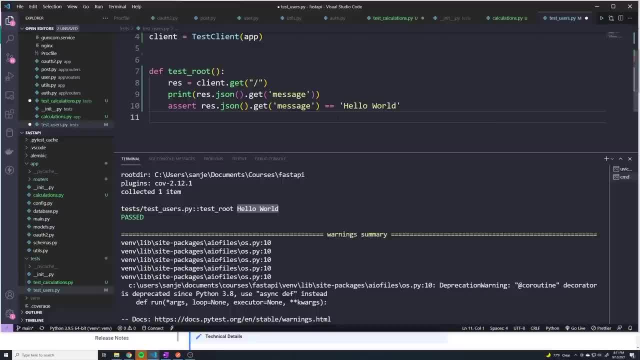 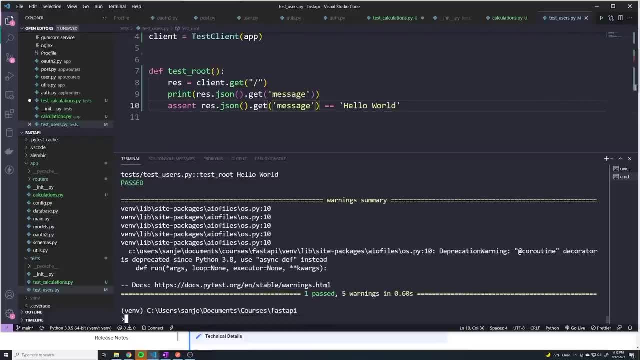 We're just performing some action, you know, running our code and then making sure that the results are what we expect them to be. And so now, if I run this again, Right, once again still passes, because It does return a value of hello world for the message property and we can assert multiple things right. 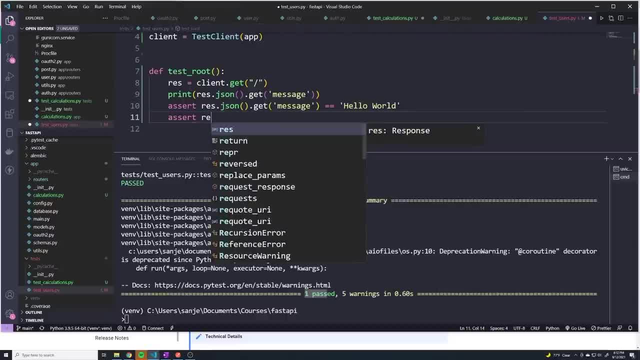 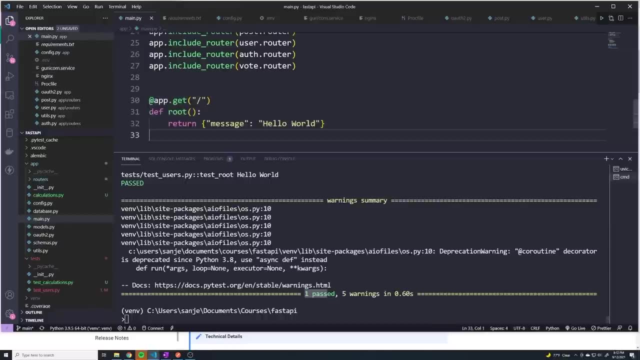 It's not just one. We can do a second test case and I can say res dot, and we can access a property called status code. It's even recommending that. so we can say: get me the status code and I could say: well, I expect this to be a. you know, if we don't change what the default status code is, it's going to default to a value of 200, as per the fast API documentation. 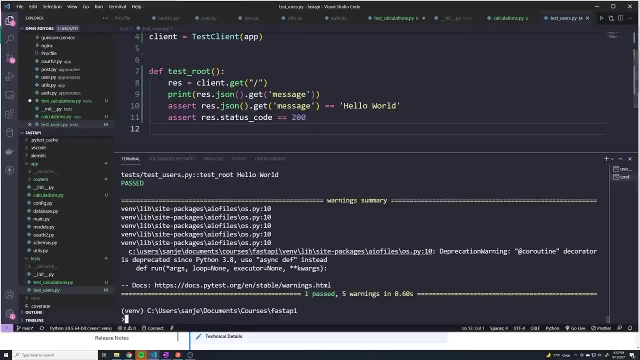 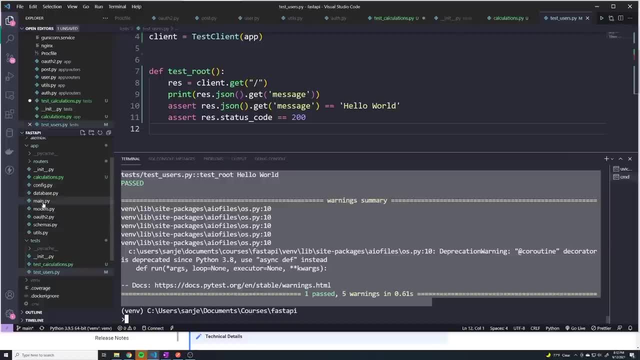 So this should be a 200.. We shouldn't get any other values. So if I run this Once again, everything works. but if I go into my code And create a little bug, let's say I just add, you know, an exclamation point or something. 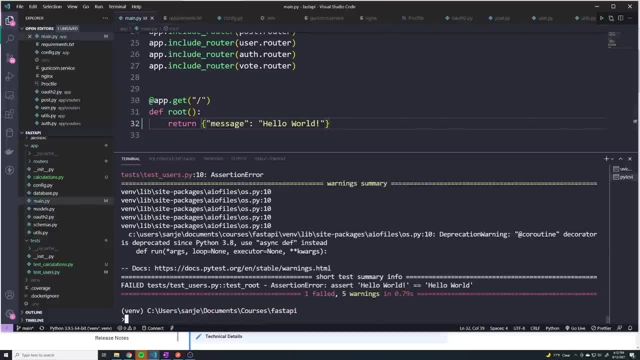 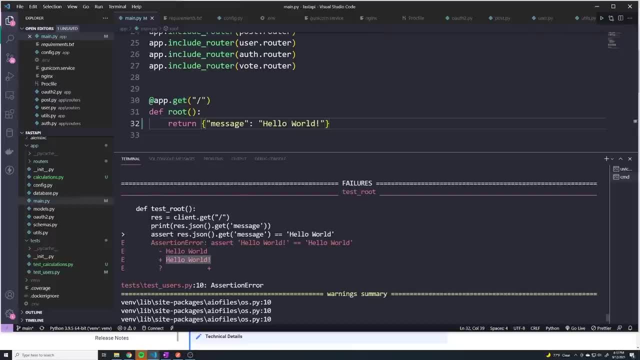 Then if I run this, We could see that it fails and that's because We expected hello world, but we got hello world exclamation. Let's change that back And this time let's create a different bug. Let's actually change what is the status code. 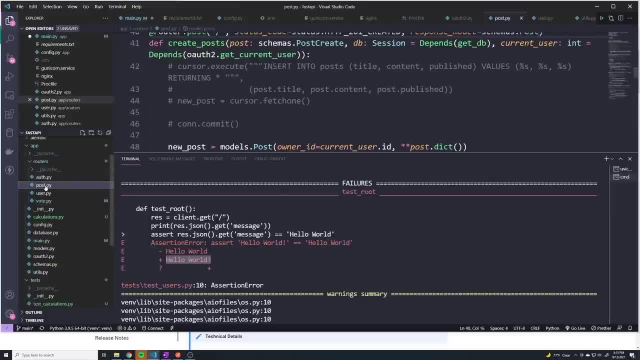 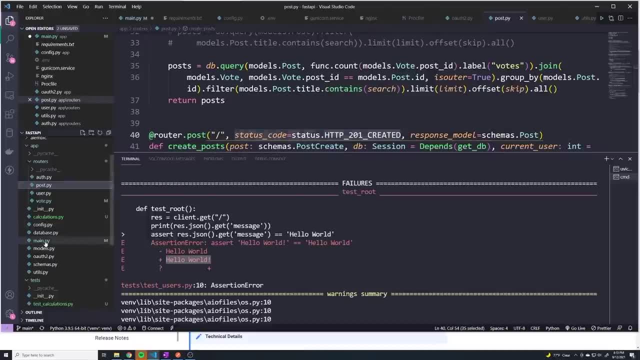 And so I can't exactly Remember how to do that. So let's go to our post router And we just set the status code right here like this. So if I copy this And go back to here- And actually was it in the decorator? 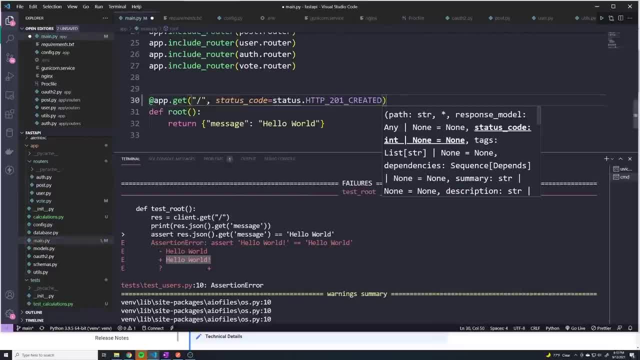 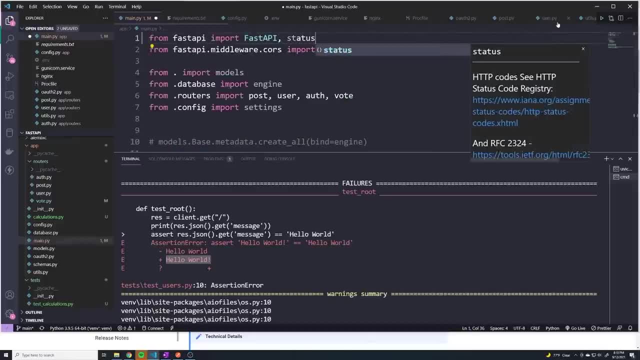 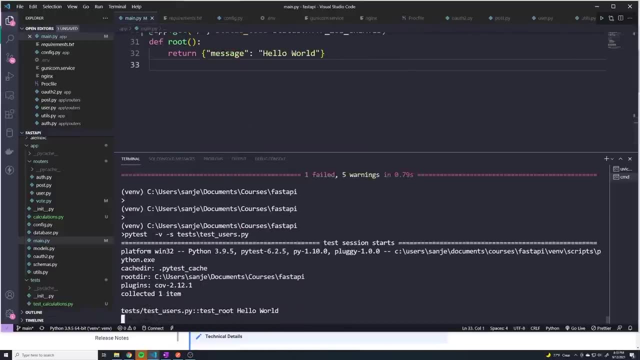 Yeah, it's in the decorator. You put that in there And we have to import status, And so now, if I try this out And run this once again, it's going to fail And that's because we're asserting, and the response was a two or one. 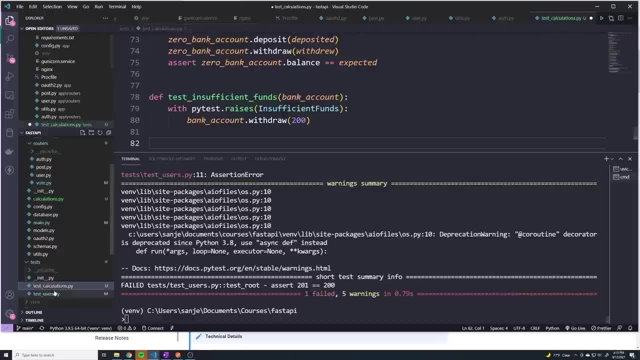 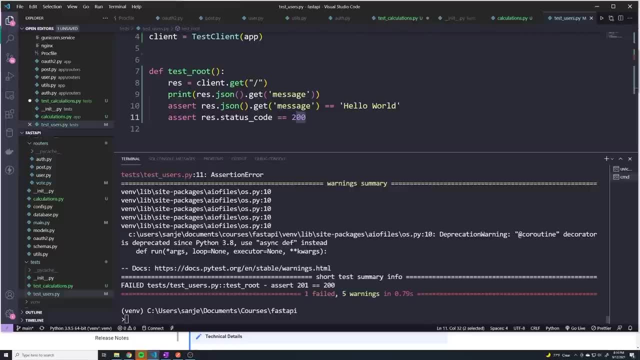 But we expected a two hundred, as per our test, which over here says it should be two hundred, And it throws an error. so you can see we could test a lot of different things. You can choose to test each and every property that you're interested in to make sure that the response is exactly what you expect it to be. 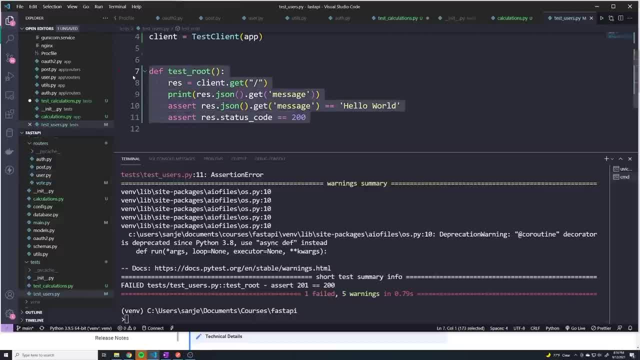 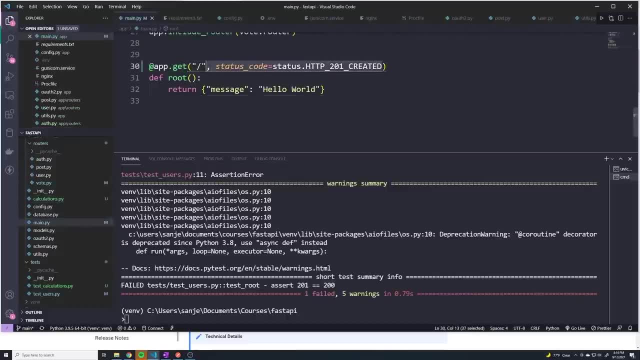 But at this point I think we understand how to send requests, So let me just first of all undo those changes that I just made, just to make sure I don't break anything else in my app and we no longer need to import that. 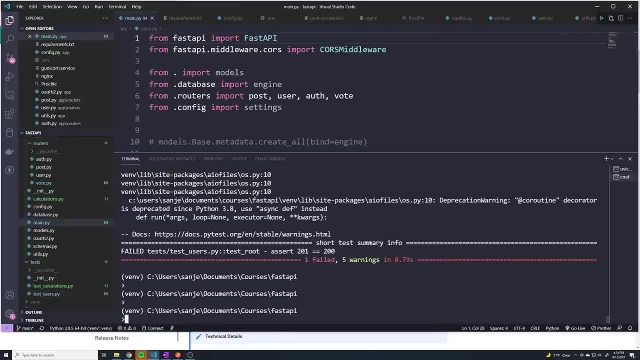 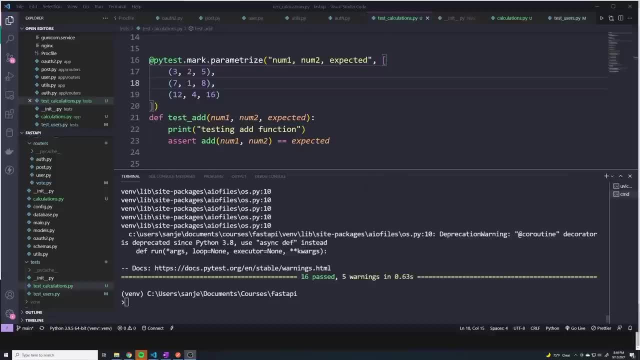 So remove that, We'll save everything, and let's just run our test one more time just to make sure that everything's good And it looks like everything passes. before moving any further, I want to show you a couple of other flags that we can pass to the PyTest command so that we can kind of tweak the behavior of our testing. 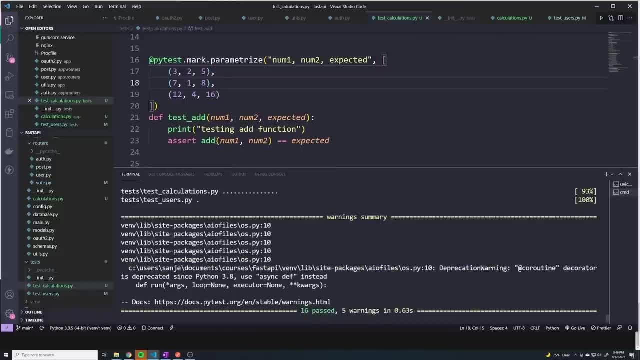 And the first thing I want to do is, if you take a look at the output, you can see that we get a whole bunch of warn And, you know, depending on how many packages and libraries that you have installed, you could potentially see a lot more warnings. 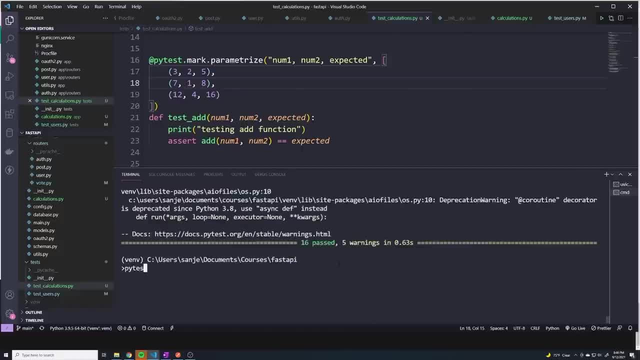 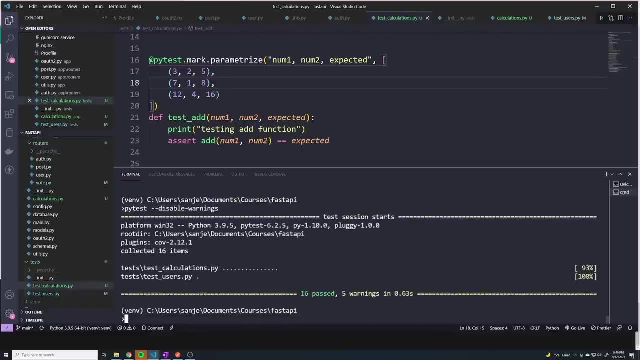 And I actually hate looking at these things. So what I normally like to do is I usually like to pass in the dash. dash, I think it's a disable warnings, I think. And so now if I run this, you could see that there's no more warnings and we just see the testing information. 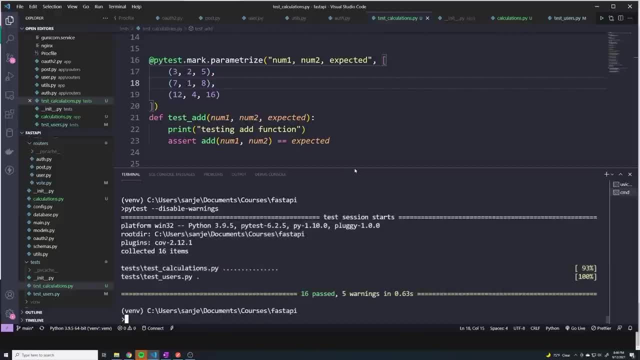 So I think that looks a lot cleaner. And then, the other thing that I want to show you guys is, until now, all of our- you know- testing, when we've broken a specific Function or class, we've only had one test fail. 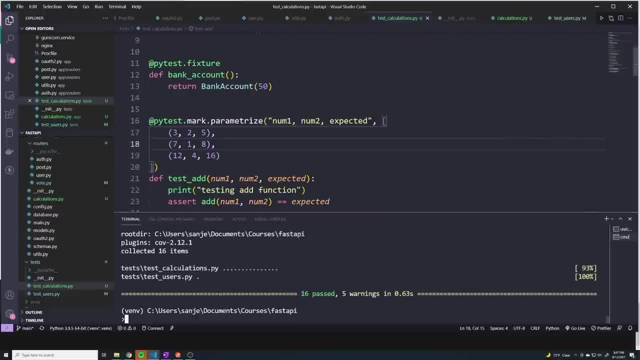 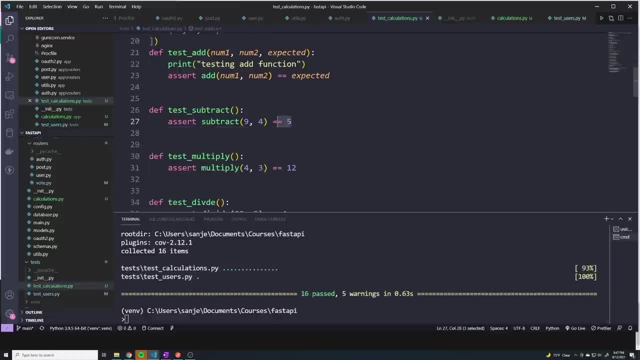 And I want to show you what happens when you have multiple tests fail. So we go all the way to the top in the test calculations folder and then maybe I just change- you know- the subtract function. So I'll change this to be six. 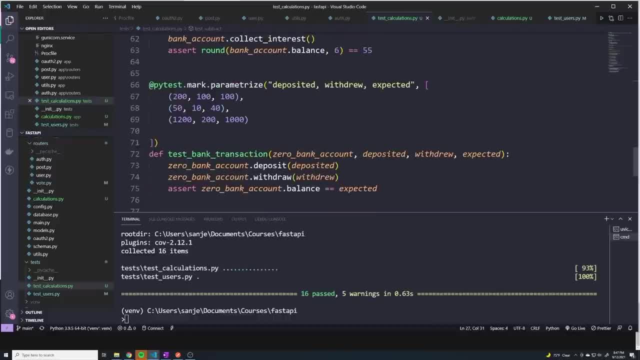 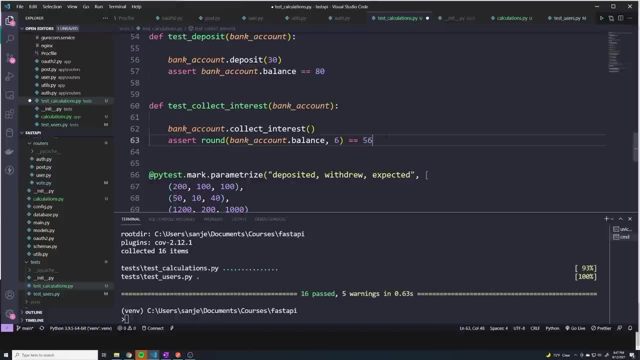 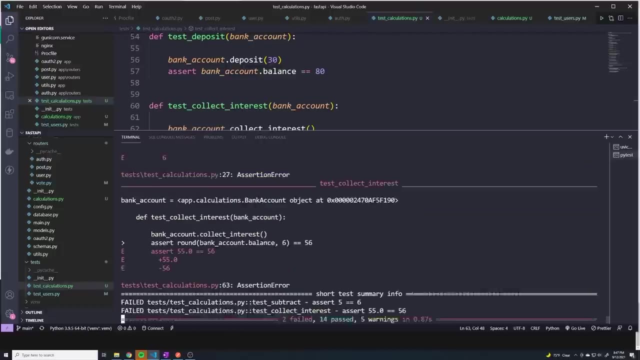 So we know that it's going to error out. And then also at the bottom, I'm going to test change this test right here So it returns fifty six instead of fifty five. And so if we run this- And I'm going to do a dash V so we can see verbose, but you don't have to do that- 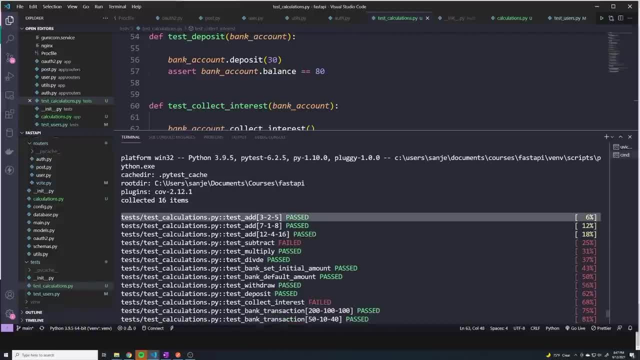 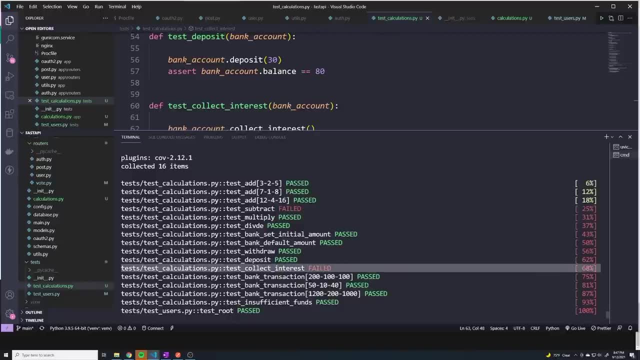 But if you take a look at what happens, you can see that you know it runs the first three tests and then the fourth test fails, and then it just continues running through all of the other tests and then it fails on the next one and then it finishes running all of the other tests. 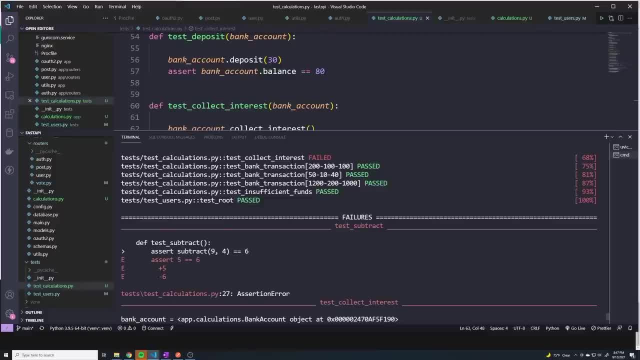 So the default behavior is, when a test fails, we're going to continue running all of the other tests, And this may not be the behavior you want. So maybe you've changed your code and you just want to see if we've broken anything. 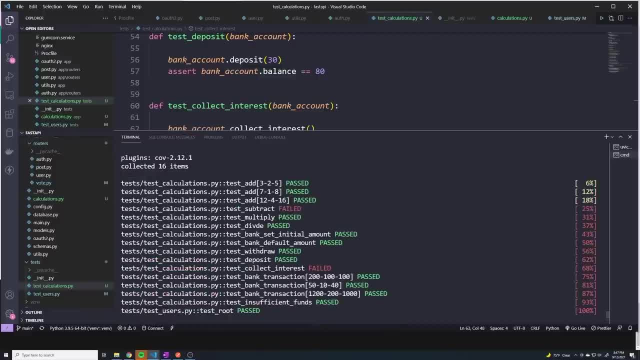 And so You want your code to ideally, you know, run through the test, and the first time it fails you want it to stop, so that you can then fix that issue and then run through the rest of the tests afterwards. Or you know you can manually run it again because you know, right now we only have like 16, 17 tests, so it doesn't take that long. 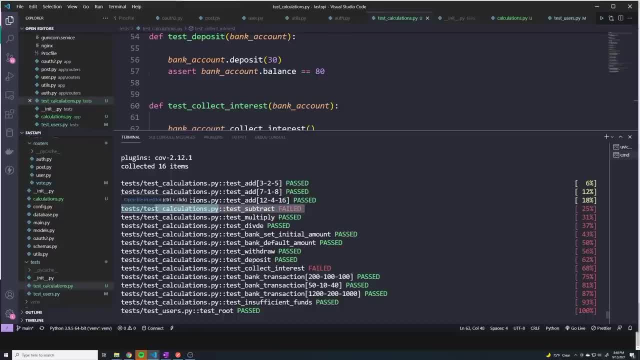 But when you start to write a lot more tests and your code starts to grow, these tests can take, you know, minutes, sometimes more than that, depending on you know. are you using an external API? Are you using a database? 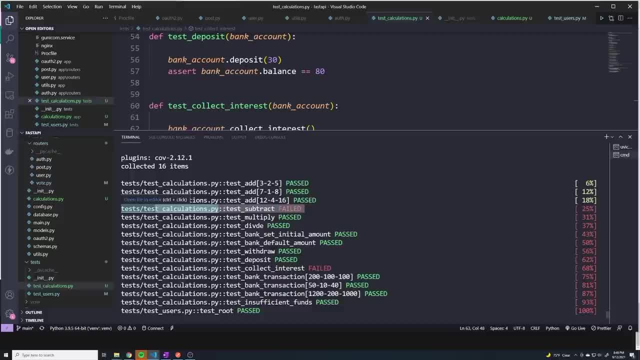 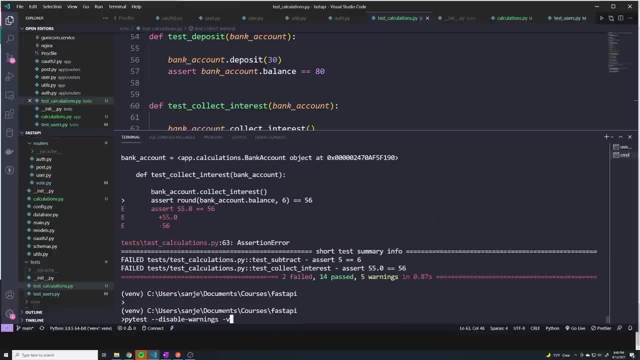 These all add a significant amount of time. If you test and if you just want to see if you've broken anything, you may want PyTest to stop on the first failure. So if you ever want PyTest to do that, all you have to do is you have to pass in the dash X flag. 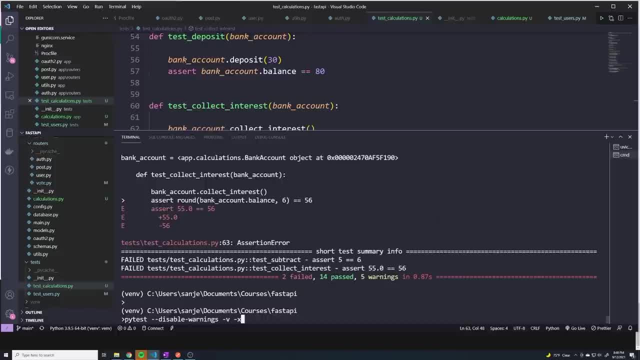 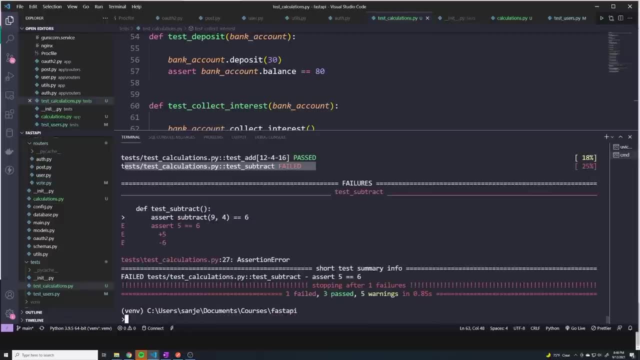 So this will tell PyTest to stop after the first test fails. So if I run this, you can see that we get pass, pass, pass, and then the first test failed and then we stop and we don't do anything else, And so those are just the two flags that I wanted to go over. 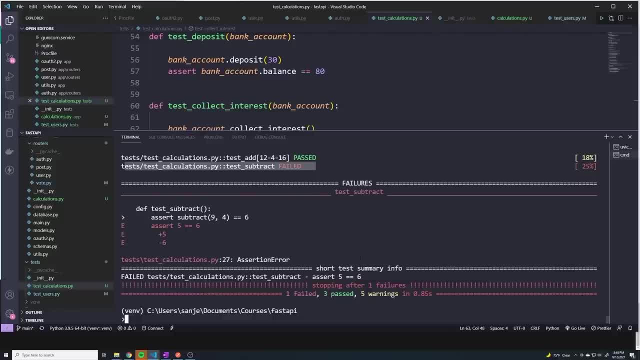 I don't think we'll really cover any other specific flags. I just wanted to go over these two because they just just happen To be two of the ones that I do like to use occasionally. But let's make sure we go ahead and change all of our code back. 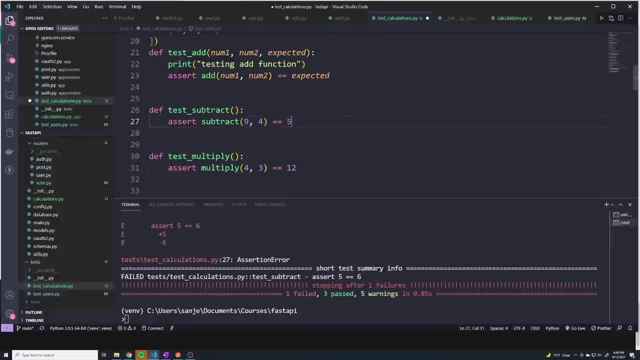 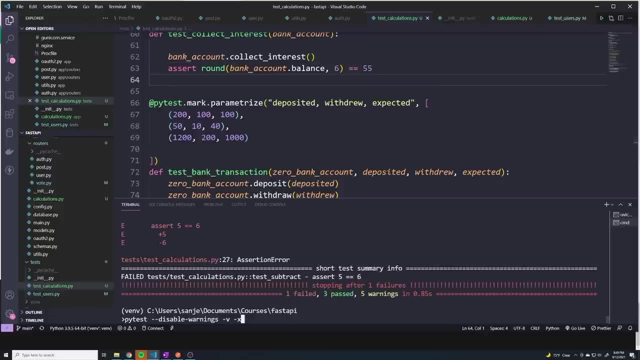 So I think we changed this one. this should be back to five And this should be changed back to 55.. And just to make sure, let's just run our code once more, just to make sure we didn't break anything and we could see all 16 tests pass. 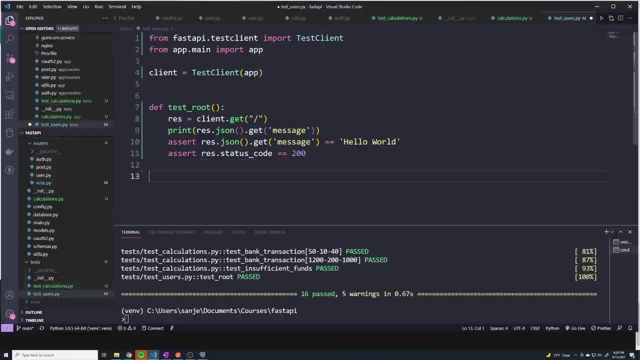 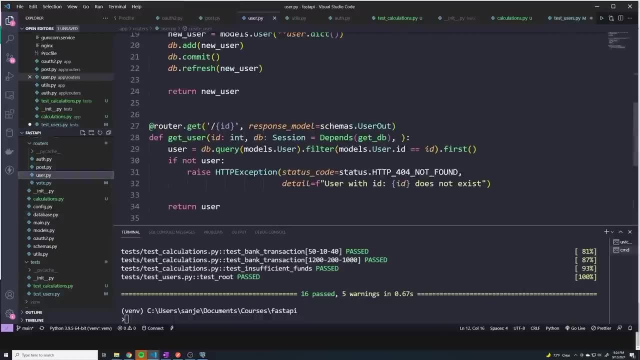 So, now that we know how to simulate a request to our API, let's create a test for testing the user, create functionality. So what we're doing is we're going to create a user And we're going to test this specific route right here where we create a user. 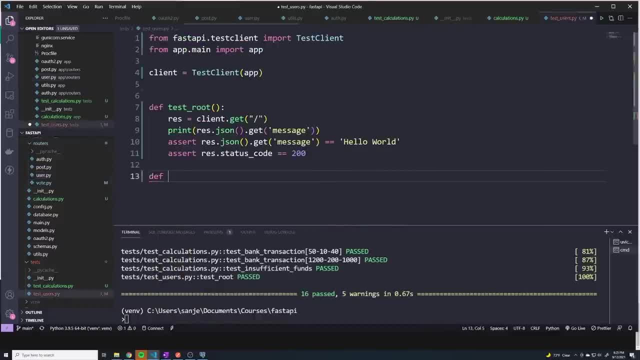 So let's try this out. We're gonna do the same thing. I'll call this a def test: underscore create. underscore user. And here I can say: res equals client, like we did before, but this time it's going to be a post request. 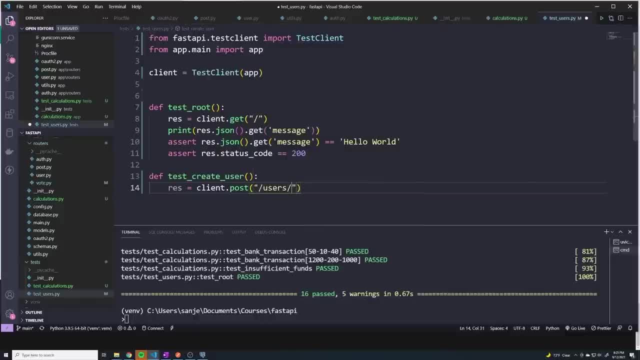 And the URL slash users. All right, and then, since we're now sending a request, you know to create a user we have to send data in the body. So to send data in the body, you say JSON equals and then you pass in a Python dictionary. 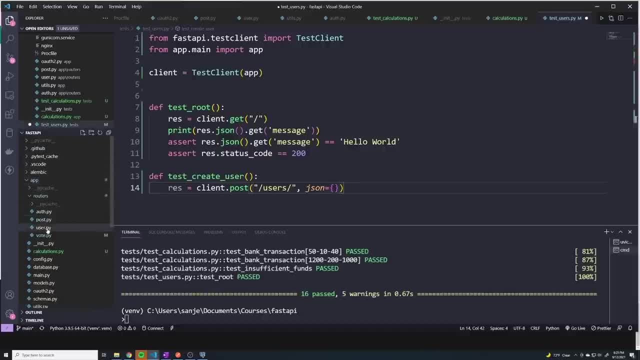 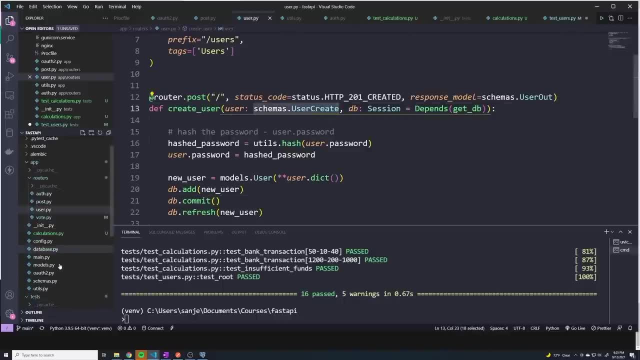 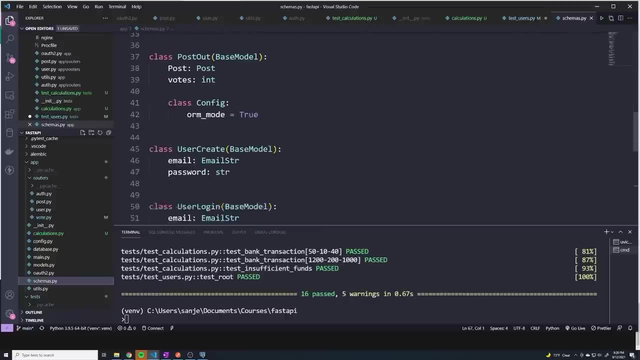 So this is going to get sent as the body And if you go back to our specific route, which is right here, you can see that we expect the users create schema. So if we take a look at the schemas, You could see that somewhere in here. whereas user create, here we go, we expect an email. 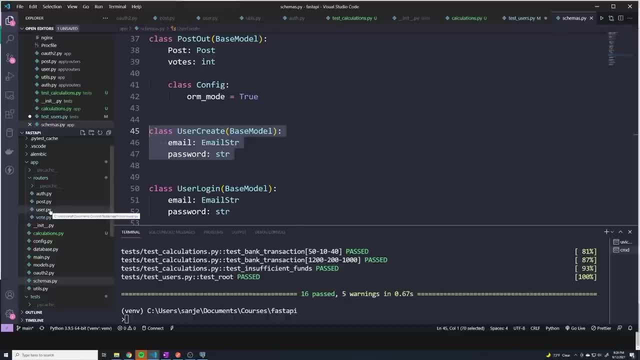 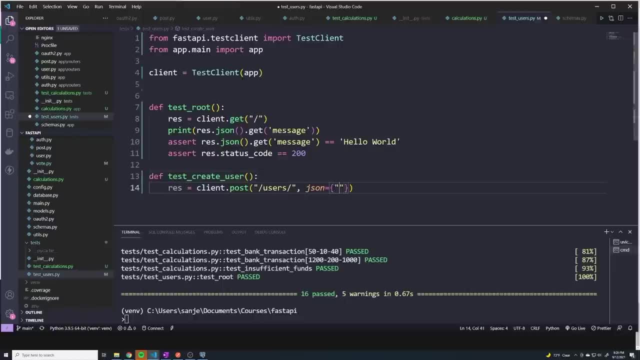 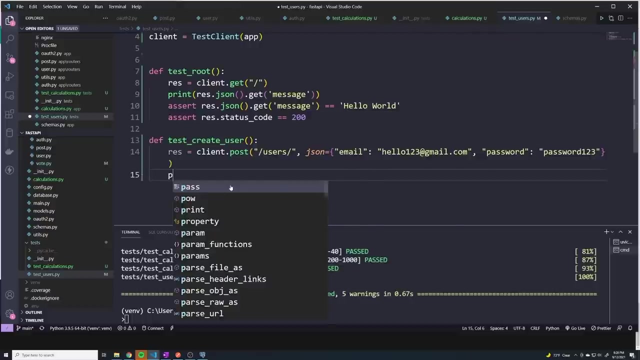 and a password. So let's send an email and a password. And so for email, we'll say: this is going to be Hello 123 at gmailcom And the password: Okay, It's going to be password 123.. And just to see that it works, let's do a print. 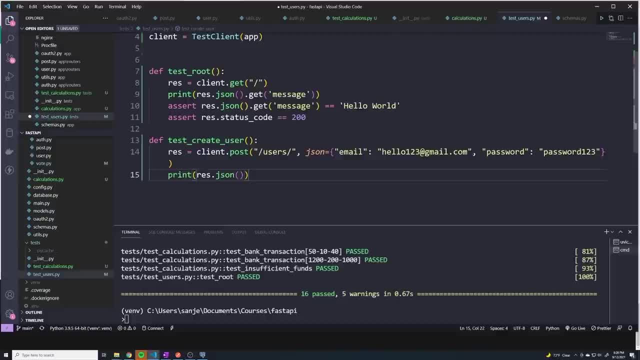 And I'll say res dot JSON, And then the test requirements that you know. how do we verify that it works? Well, let's start off with something very simple. So we'll say assert And I'll say res dot status code. 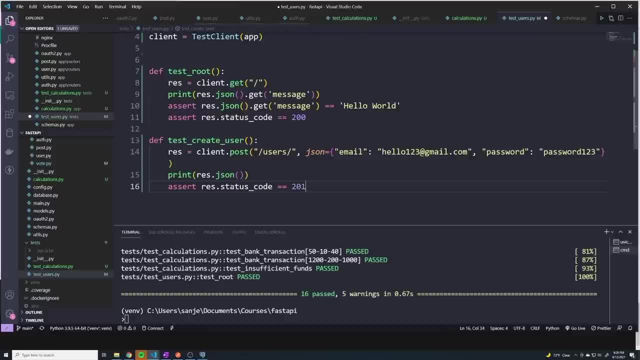 We know that when we create a user, we expect a 201.. And we can just verify that by taking a look at the code. It's a path operation, But I think this should be good. And then now, if I run this, I'm going to run just this file. 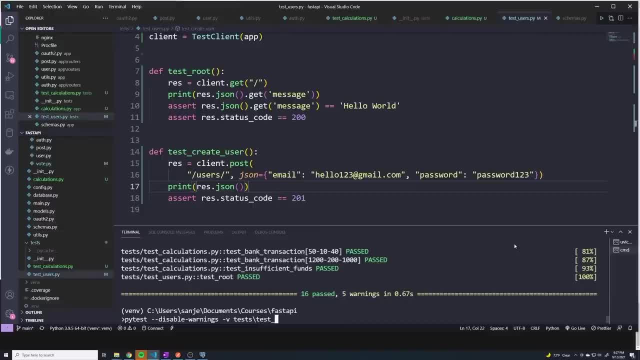 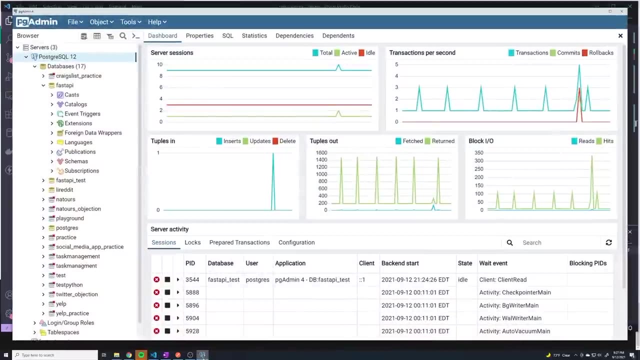 So I'll say test, test user, And let's see what happens. So we see both of them passed. And how do we verify that? Well, I mean, if we should see this user in our database, right? so if I go to my PG admin, 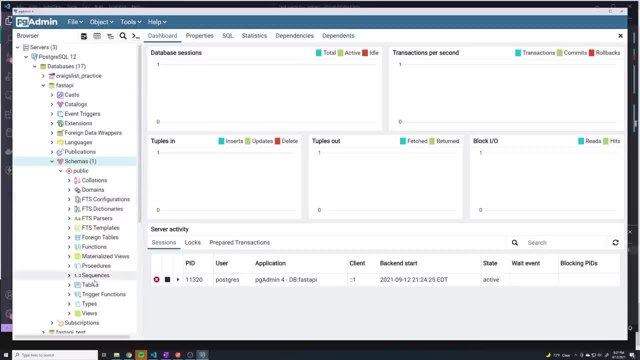 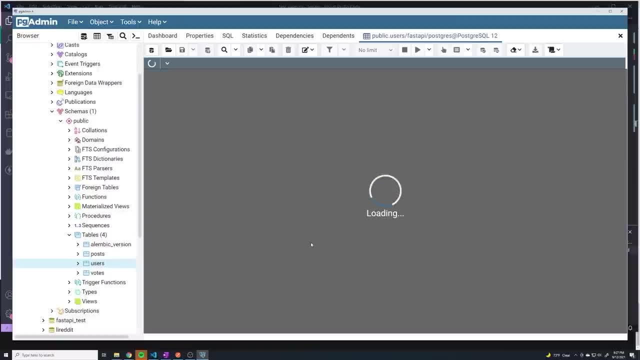 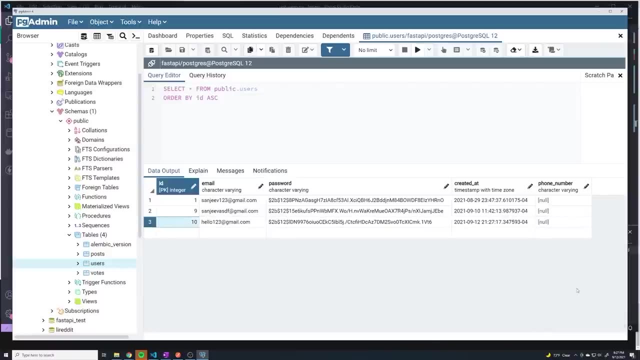 go to my database And we'll go to our schemas tables and go to users and we'll do a view at it all. We get to the Hello 123.. So it was successfully created. I'm just going to quickly delete this again. 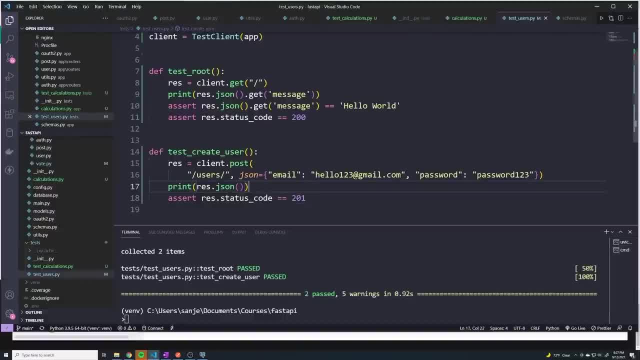 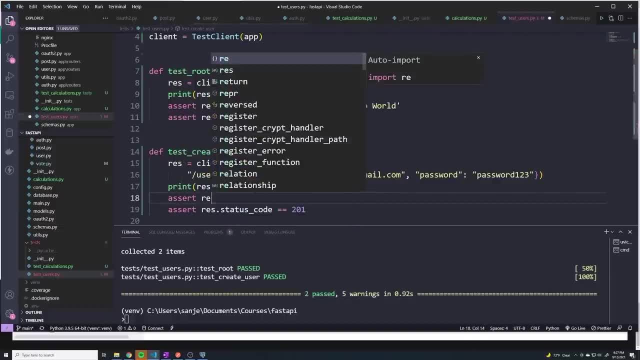 Well, actually, let me show you what happens if we don't. I'm actually going to do something unique here. I'm going to say: well, actually, let's just do an assert And I'll say res dot, JSON. 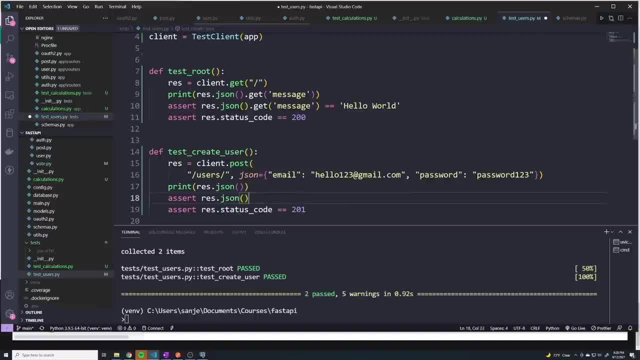 Okay, Okay. So I'm going to go to JSON dot get And we want to get one field just to verify that it's correct. So what's the data going to look like when it comes back? Well, we should see a print, but I didn't. 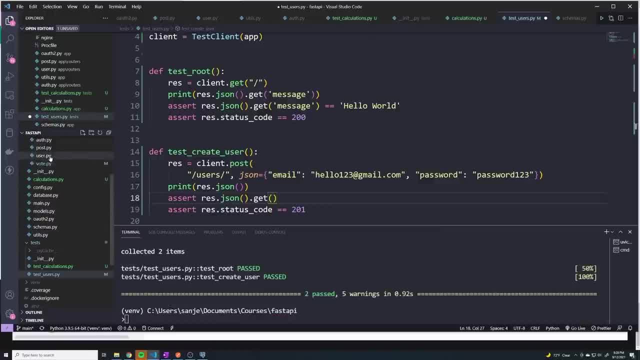 That's because I forgot to do the dash s flag. But, going back to the route, we're going to send the response as a user out, So we expect it to match this specific, this specific model right here. So it should have an ID. 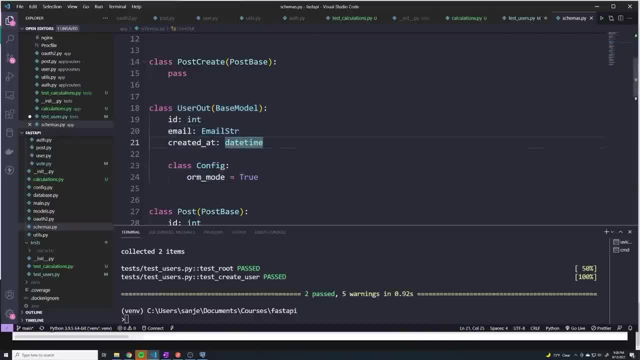 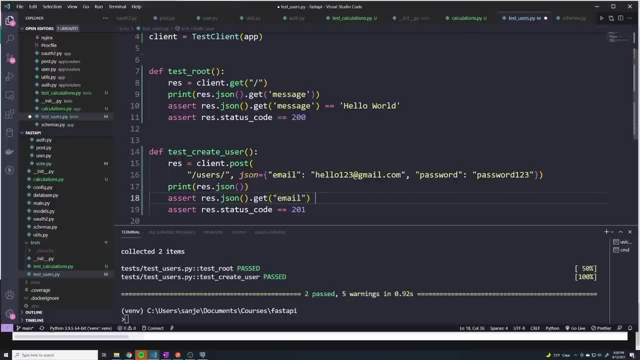 Okay, An ID, an email and a created at. So let's add that in there. I should expect the email to equal- equal the email that I gave it, And you can really do as many you know asserts as you want. 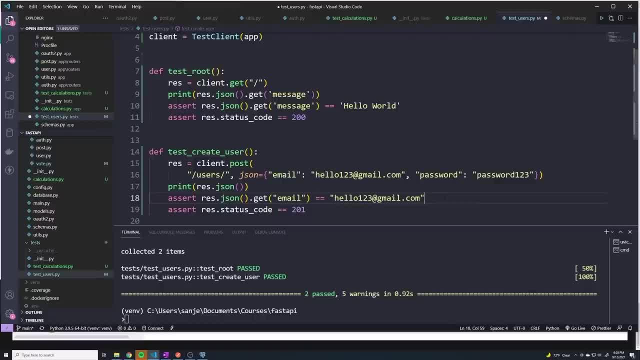 So you can verify each single property has been set. you can verify that an ID has been set. I'm just going to keep it simple. we'll just say just the email, we'll just run that check And so we'll run it again. 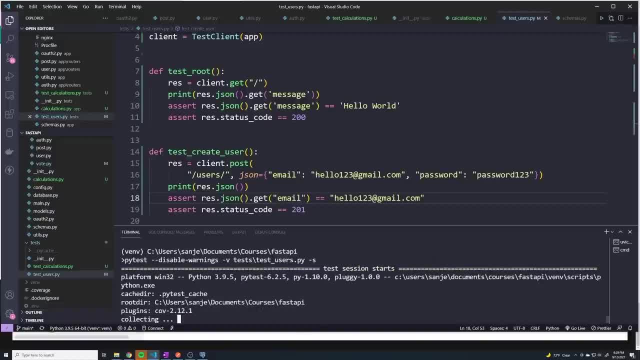 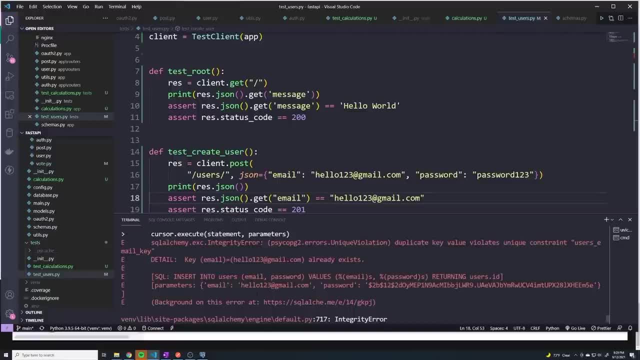 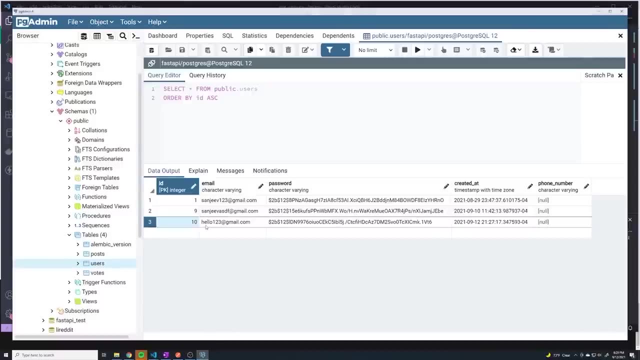 And I'm going to do the dash s flag as well. All right, and we see that it failed, And we can see that it failed because there's a duplicate key, violates unique constraint of email, And that's because this user was already created. 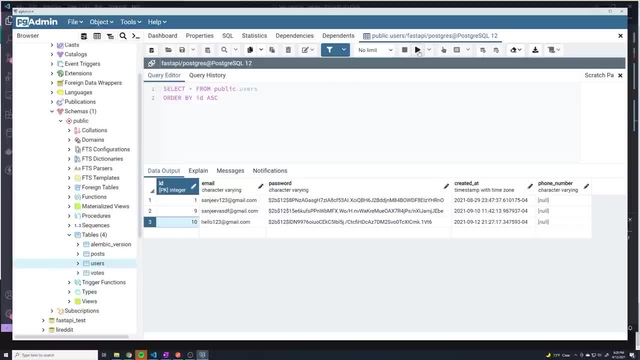 So I can't recreate him. So let me delete this. And I don't think I. Yeah, If I select the number and then go to: Oh no, it doesn't look like I can, Here we go. Now I, once I select that number, I can delete this user. 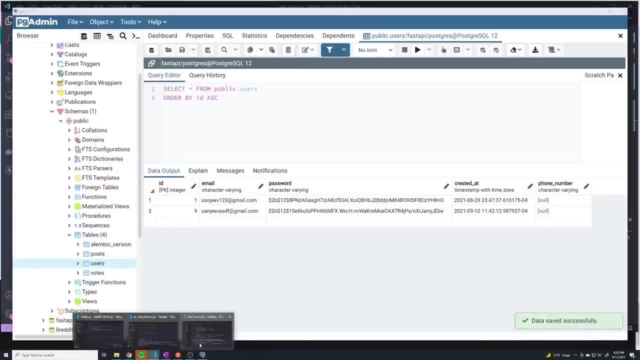 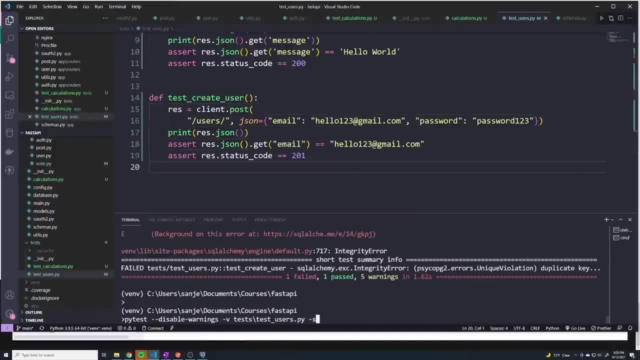 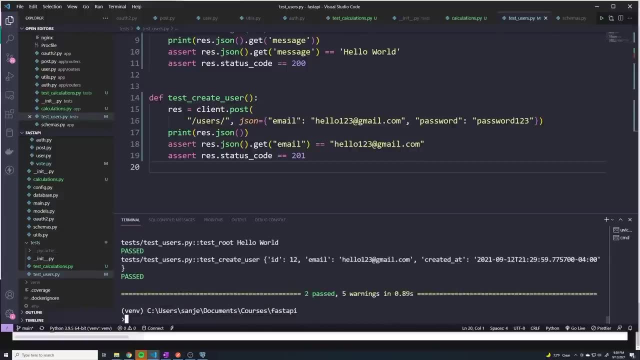 And then we could save that to database. And so now, if I run this again, we should see it work And we can see that both tests pass And we can see that both of our assert statements were checked and validated and they both 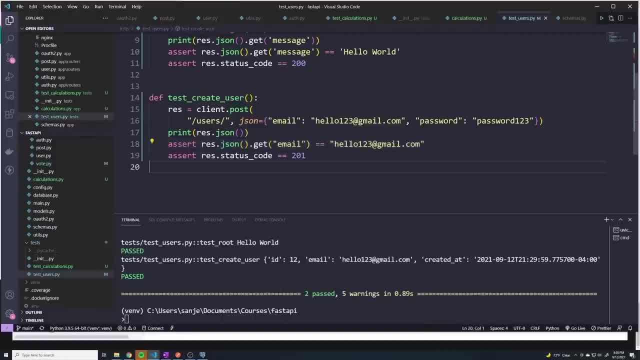 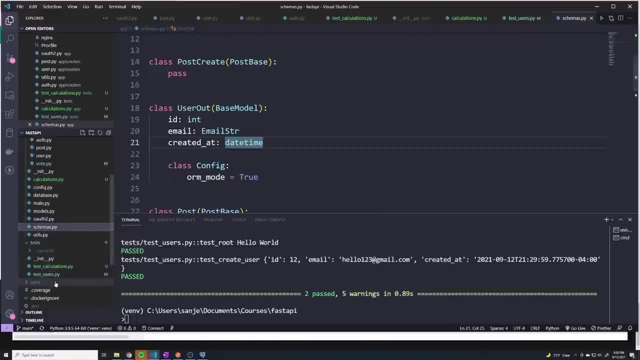 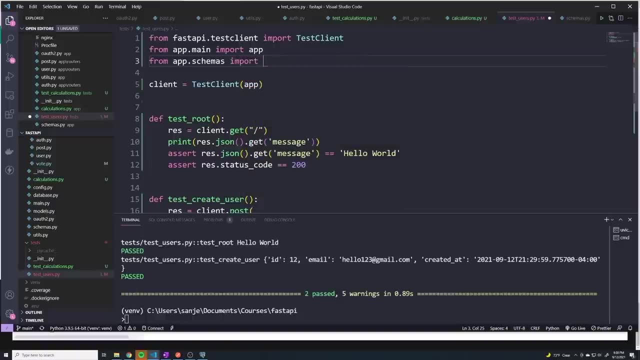 looked good. But instead of doing it like this, we can even take it one step further. Instead, what we can do is I can actually import this user out schema into my test, So I can say from app dot schemas, import user out, and then I can remove this print. 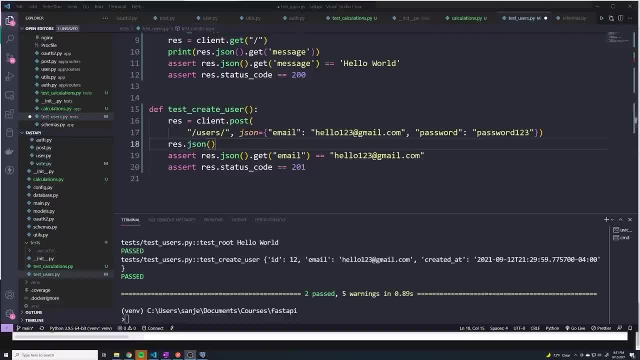 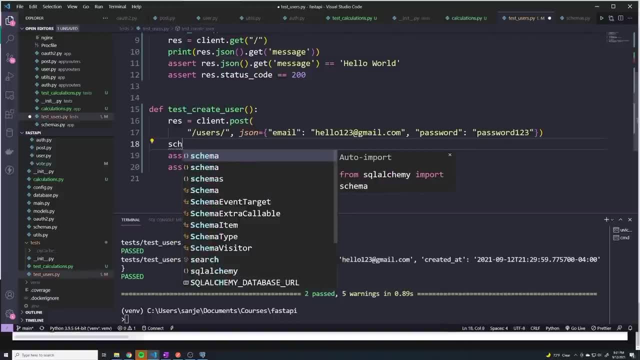 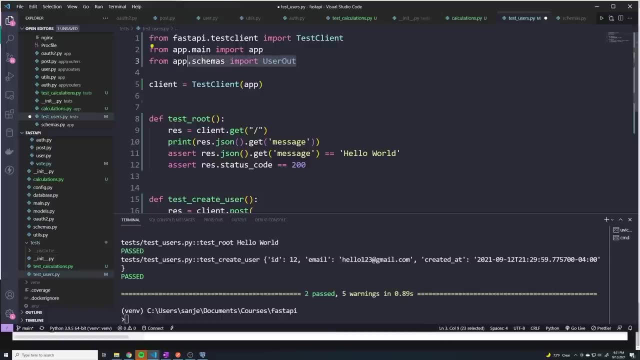 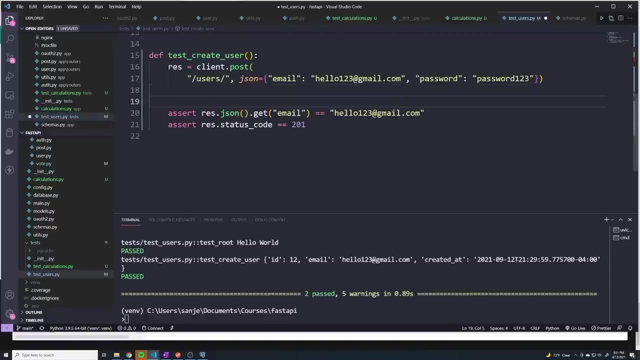 statement And what I can do is here I can actually use the schemas. Actually, sorry, I'm actually going to change this import. I'm going to just import all schemas, So say, from app import schemas, And now I can actually create a new pydantic model and I'll say: schemas dot, user out. 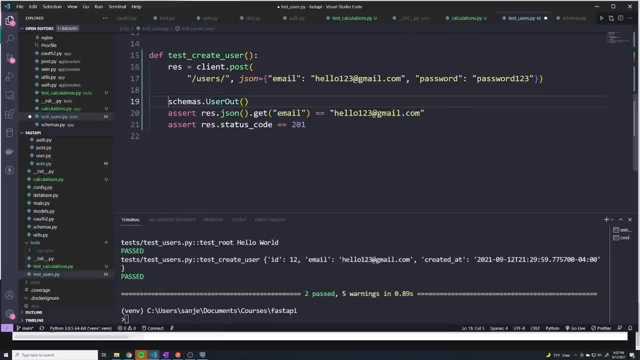 So we're going to create a new schema And I'm going to save this as a variable. I'll call this new user And we can pass in the data that we get back from the response so I can say res dot JSON. 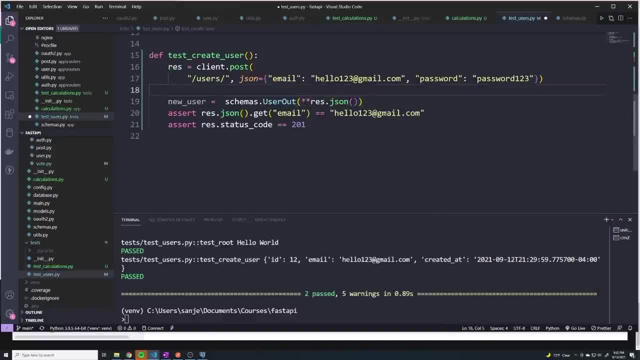 And remember we have to actually unpack the dictionary. So it's in the right format to create a new user out model. And now this is going to perform a certain level of validation. So it's going to confirm: hey, do we have an ID? 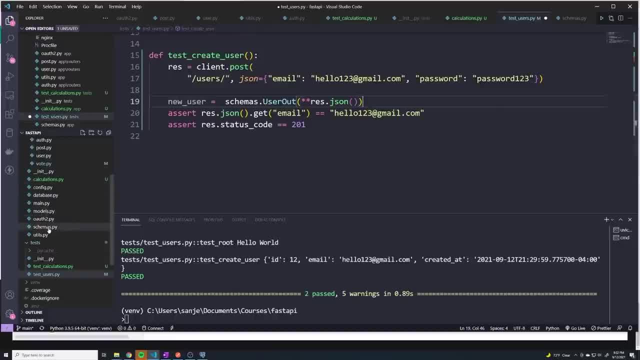 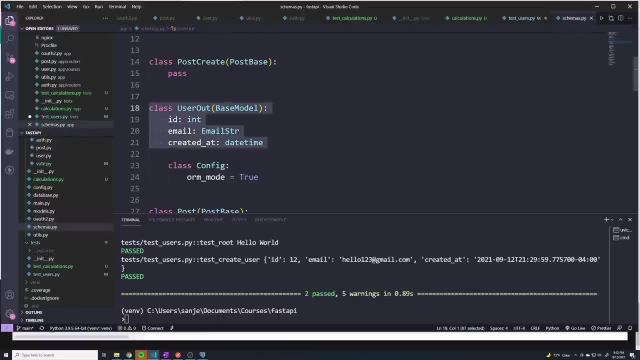 Do we have an email? Do we have a? what was the other thing that we needed? And do we have a created at? so it's going to make sure it's got these three things. it's not going to check to make sure that it's the right email. it's not going to check. 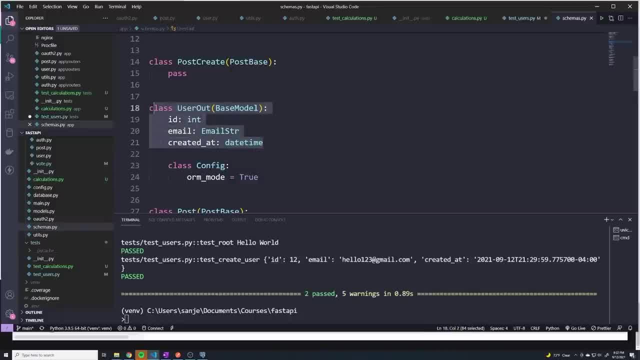 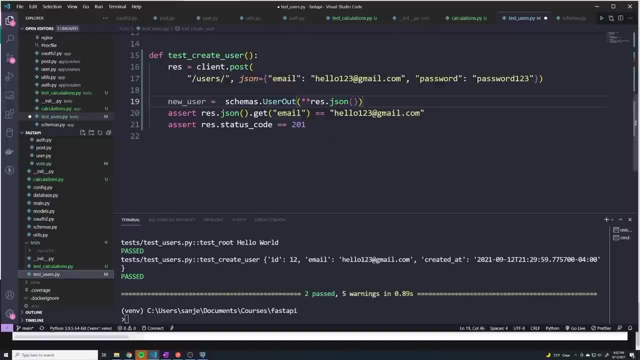 to see if the right ID, but it's going to check to make sure that at least it has the three properties. So it automatically does some of the validation for us And it'll throw a an error if one of those are missing. And if it throws an error then obviously pi test will consider this test a failure. 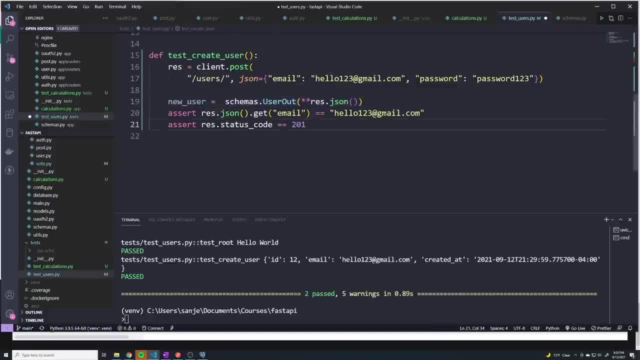 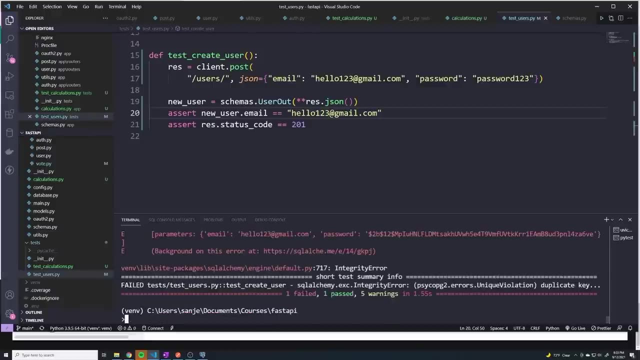 So by doing this we've kind of we've kind of saved us a little time, And now I can actually change this. instead of doing this, I could say: new underscore: user dot. Email equals this value. So now, if I run this, hopefully this works. 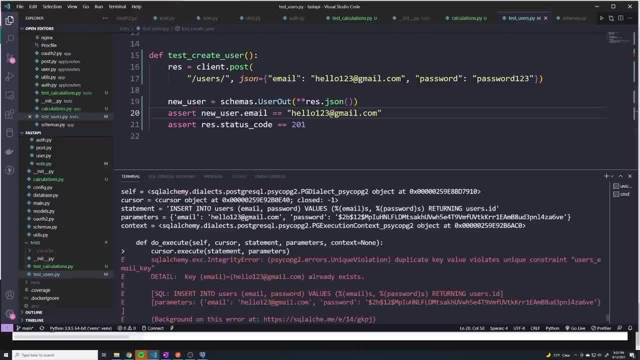 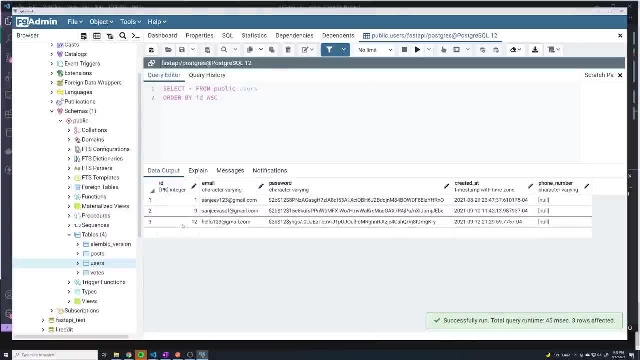 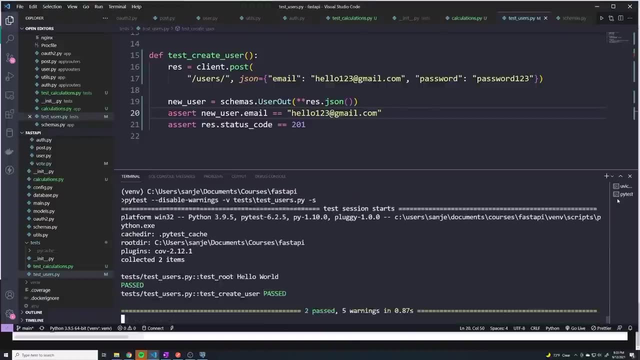 And it looks like it failed. And let's quickly see what happened here. Oh, once again, I forgot to delete the user beforehand, So we'll delete him and then try this test one more time. And they passed. So I think this is what we're going to do: moving forward, we're going to make use of 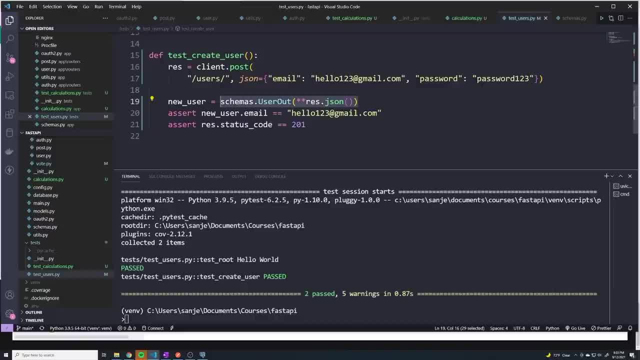 our pydantic models to do some of the validation for us automatically, so that we don't have, like you know, 60 or seven- probably not 60. But we won't have 510 different assert statements, which you can absolutely do. 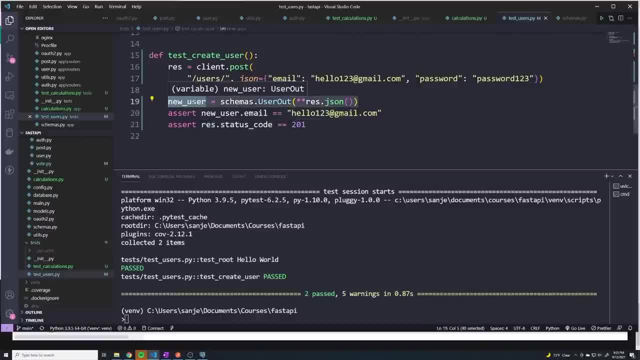 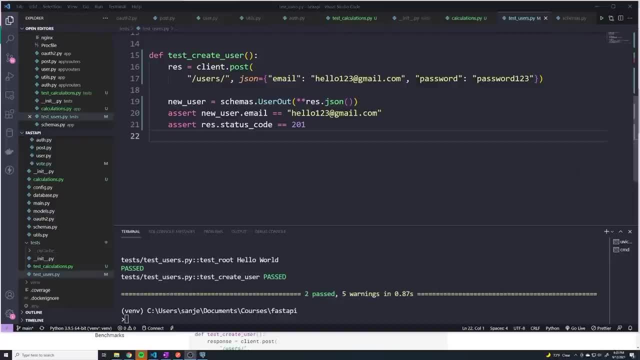 And you probably do want to, but this will remove some of them because it's at least checking to see if some of them are there. So, before moving any further, you know we need to address something important, And that is that right now we are using our development database for our tests. 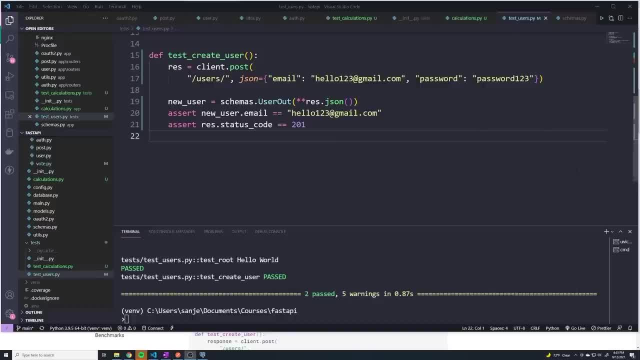 And that's not good. I don't want to use my development database. I want to create my own separate database to perform testing on, so that I don't get in the way of development or staging or any of our production databases. I want to create a completely separate database for testing. 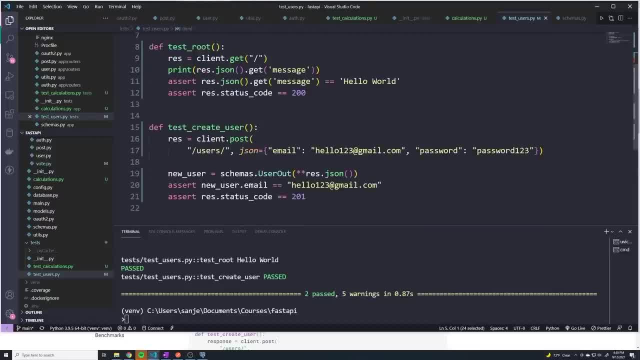 Right now, when we, you know, import our client right, we're going to be using whatever the database is that we've defined in the rest of our app, which is going to be our fast API database within PG admin, And we can see that right here. 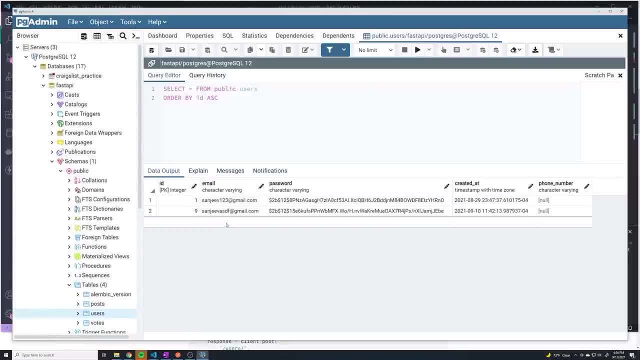 And so that's why I'm having to go in, And so that's why I'm having to go in, And, you know, make sure that it's created, and we've already got some other data which could potentially break our tests. 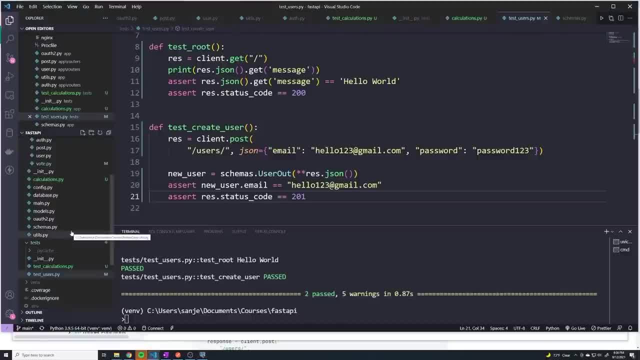 And so I want to make sure that we have a completely separate database for testing, so that it does not get in the way of anything else. So how exactly do we do that? Well, one of the great parts about the way we've set up our database is if we actually 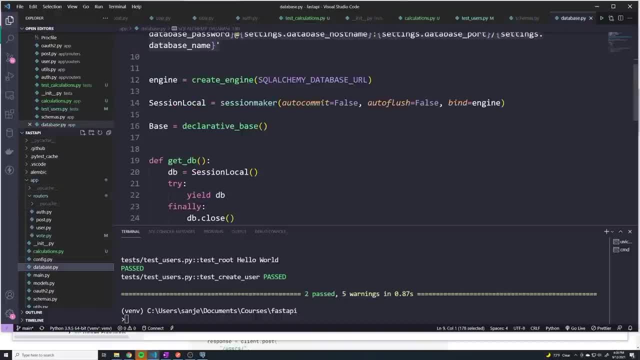 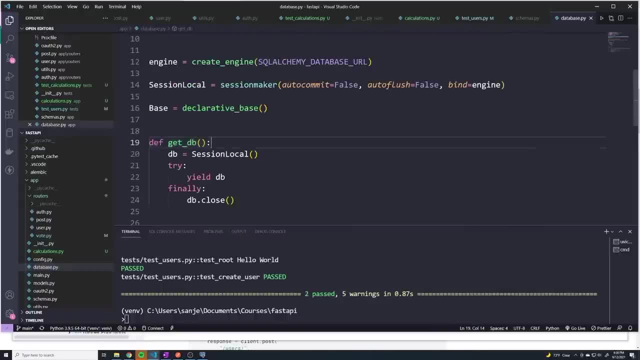 go to our database dot p- y file. right, you could see that we've actually set up a date, a dependency. So when we set up our dependency, you can see we created this function called get DB And this get DB actually returns the set. 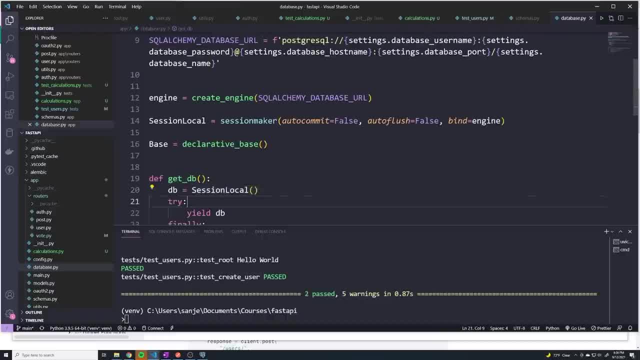 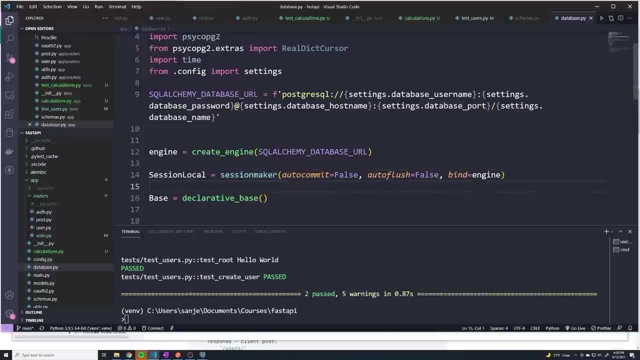 And this get DB actually returns the session local. So this is what allows us to actually, you know, make queries using SQL alchemy, And that comes from this, right here, from the session maker, where we passed in all of our database connection details. 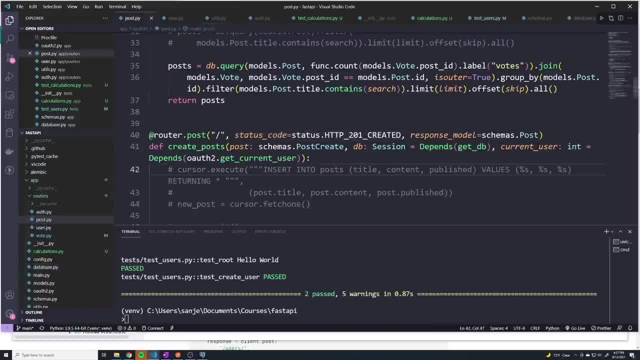 And if we go into any one of our routes- it doesn't really matter which one- you can see that we pass in the dependency into the route. And the great part about having dependencies is that it's very easy to override a dependency in any environment, especially a testing environment. we can say hey, instead of passing in you. 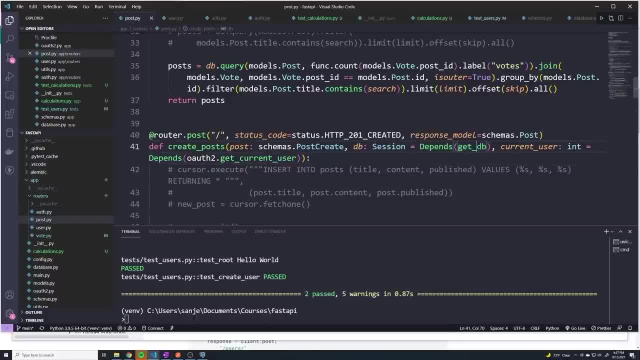 know, get DB. we can say: you know something like get, I don't know. underscore test, underscore DB, which is going to be a function that returns a test instance of our database instead of our development instance of our database. 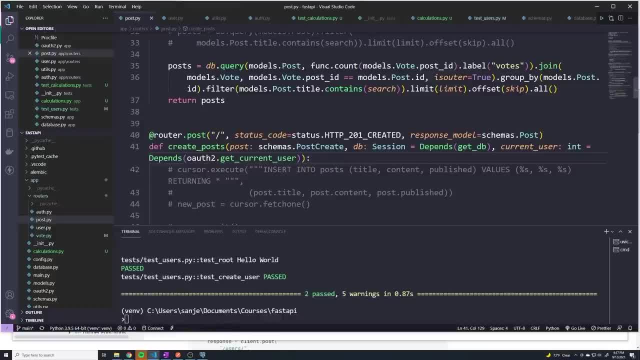 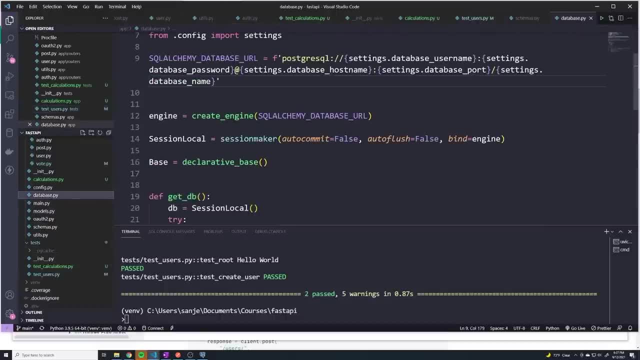 So I'm gonna show you guys how we can set that up and how easy that is. So we'll go back to our test users And we're essentially just going to copy all of this right here. So I want you to copy this all the way up to the URL. 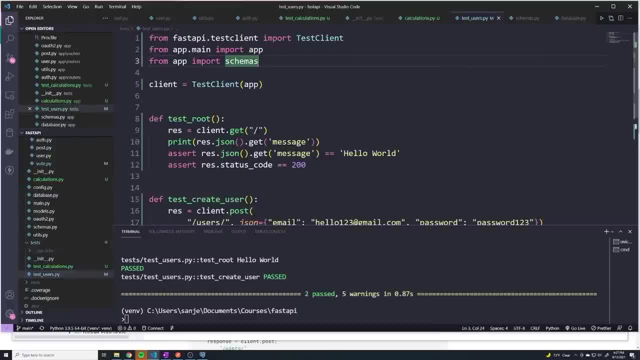 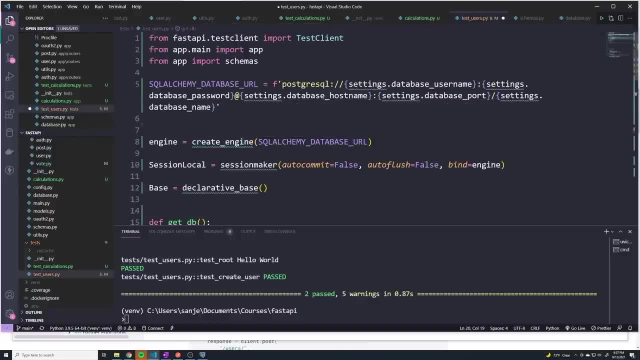 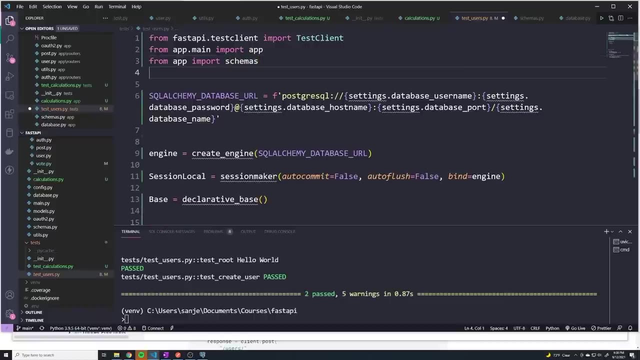 And we'll have to set up some imports, And we'll come back to that in a second. So let's just create some space, Alright. so we've got all of this and we need to import a few things, So we'll start off by we'll have to import settings. 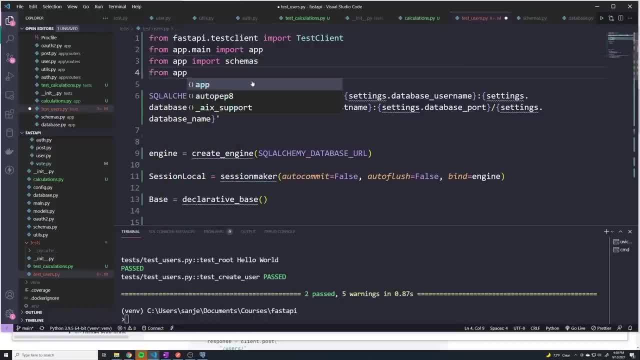 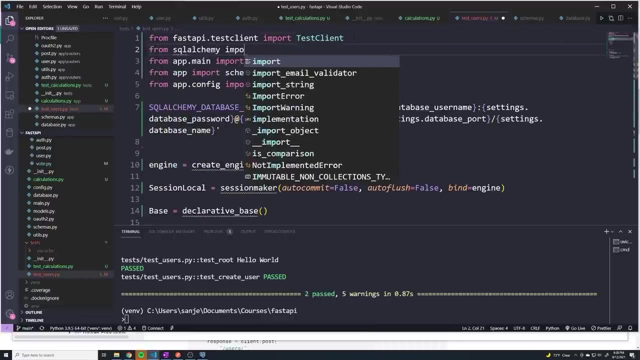 So we'll say: from app import. actually we'll say from app dot config import. I think it's settings Yep, Alright, so we've got that cleared. We then have to import, create engine. And so we'll go up here and I'll say: from SQL alchemy import, create underscore engine. 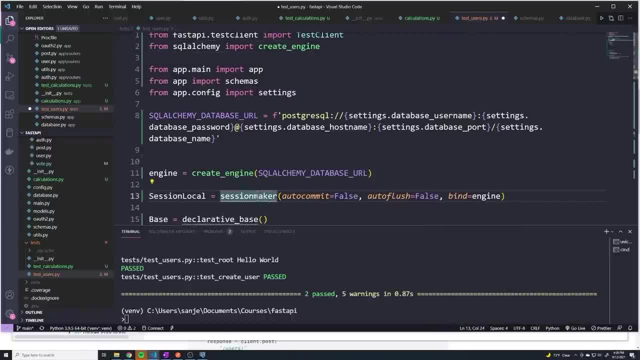 And then we need our session maker as well, And I think if I hover over this can I know if it doesn't look like it'll auto import that for me. So I'll say: from SQL alchemy dot ORM import session maker. 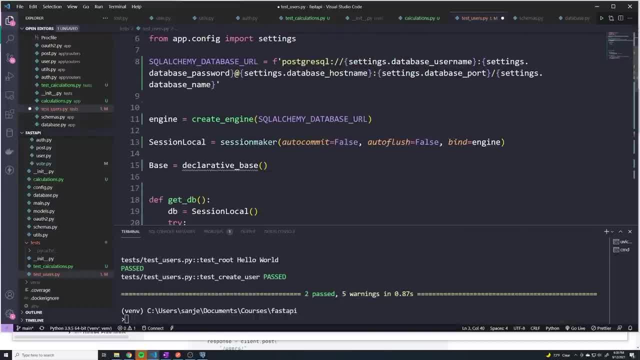 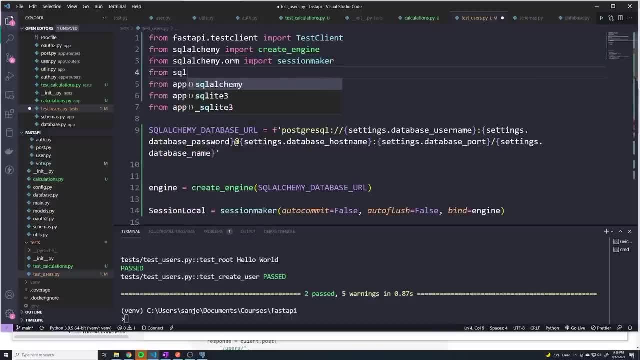 Alright, it looks like we got most of the issues We still need to import. We'll need declarative base And we'll import that. I'll say from SQL: alchemy, dot, ext, dot. declarative import, declarative base. 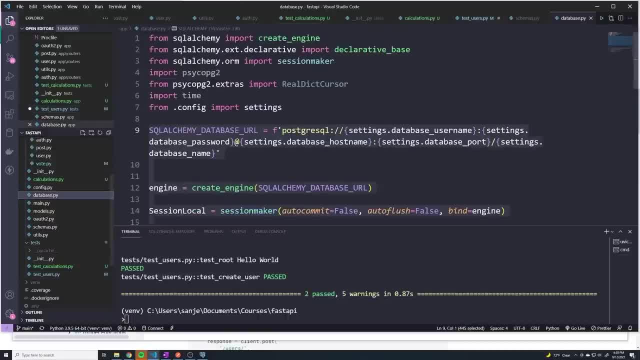 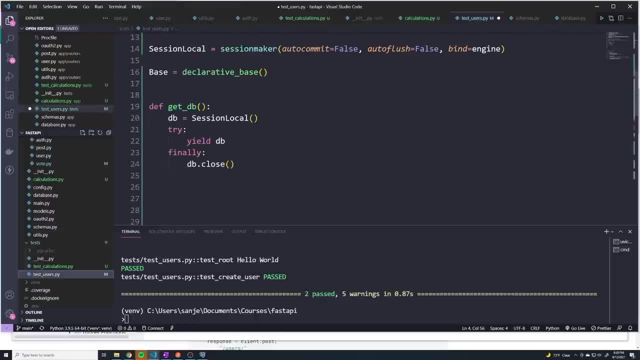 And if you guys don't know where I'm getting this, I'm literally just copying this straight from this file. So everything that's here, I'm just you can just copy it as well, And if we go down, I think we have everything right. we no longer have any errors. 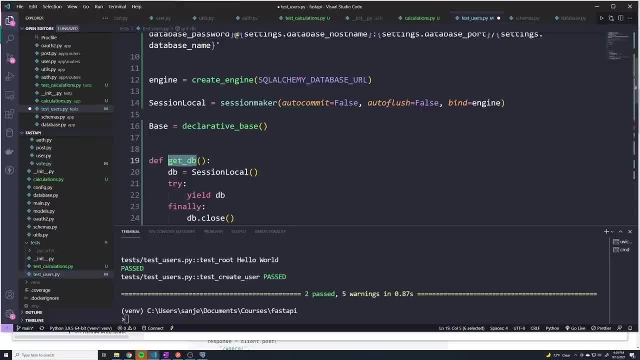 So we've got all of our imports, And so this is the function. This is the function that returns our session local. So this is what allows us to query the database. This is our session object, right, And this is how it's set up exactly in the database. dot p- y file. 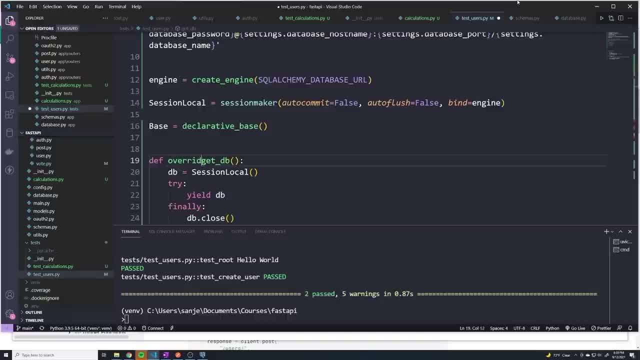 So what I'm gonna do is I'm going to create another function, but this time I'm gonna call it override underscore, get on score DB, And this is going to return this session local instance. But I'm going to rename this just so I don't get it confused. 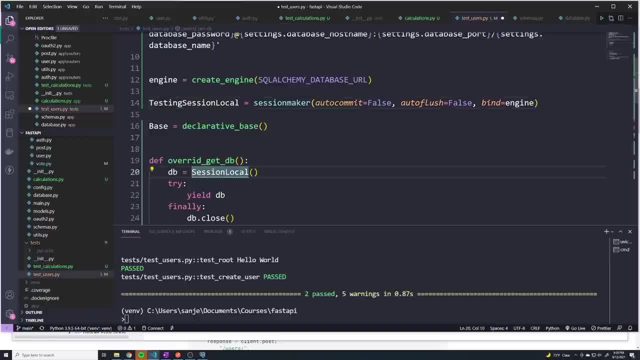 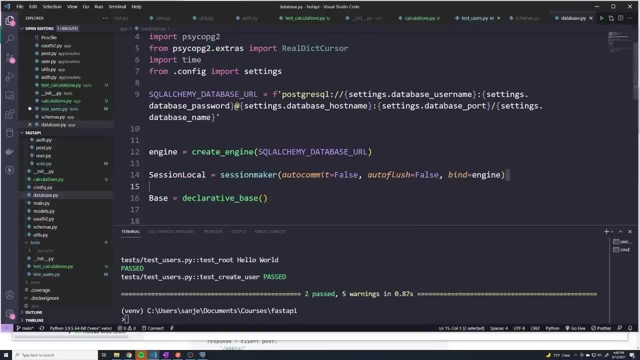 And I'll call this testing session local, Okay, And then I'll reference this All right. And so that means right now, in our current application, we're referencing the one that we created in our database, dot p y file, But the one in our test we're going to actually make use of this new one right here. 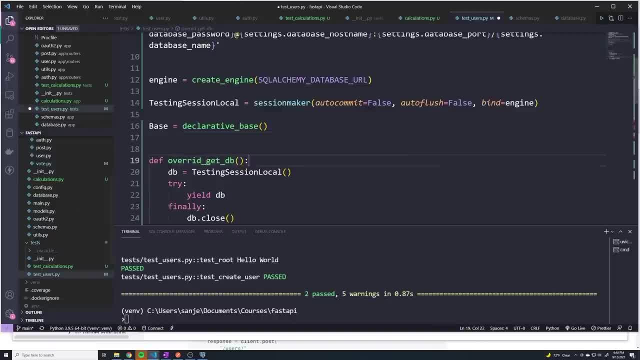 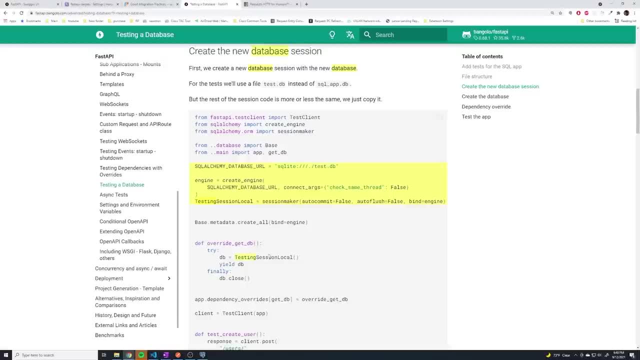 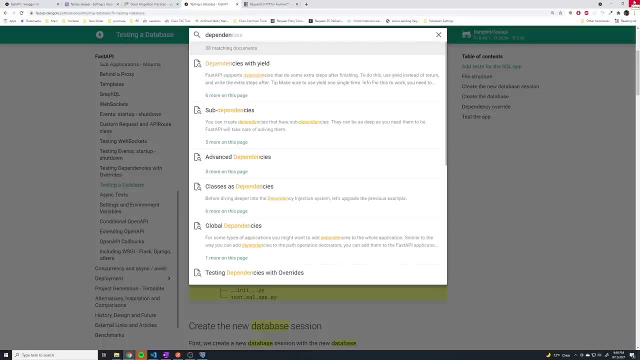 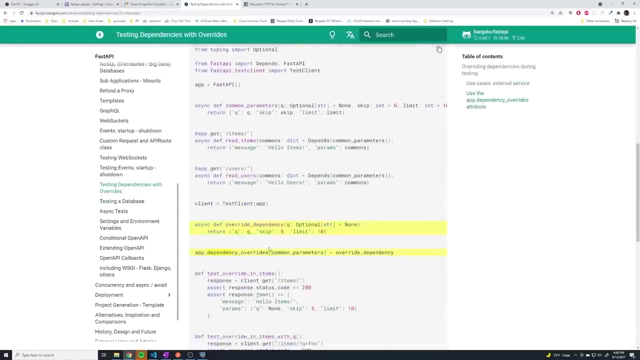 If we call this override, get DB. So how exactly do we override the database or any dependency? Really Well, fast API has a section on here And I think if I search for dependency Testing dependencies with overrides to actually set up the override, you just do app dot dependency. 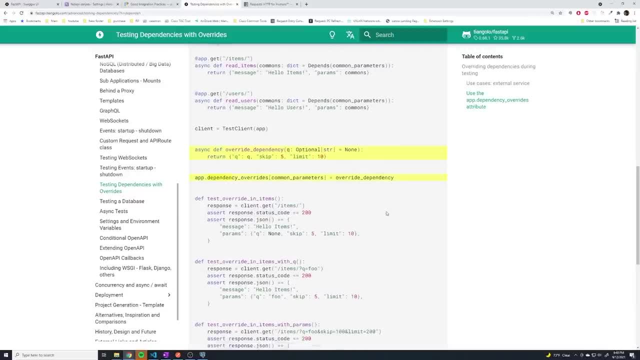 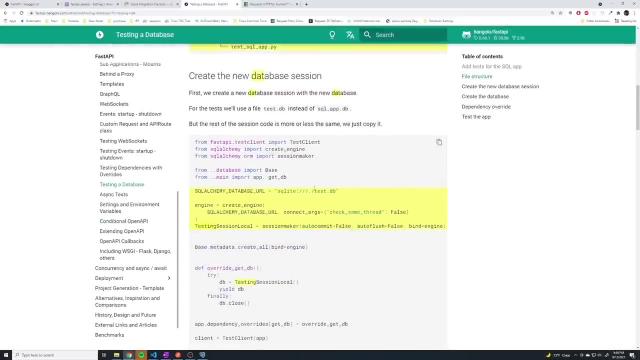 override And then you provide what you want to override it with. And there's actually a better example. if I go to testing database, this will actually show you how to do that. So we've got the override DB where we've created a different session object. 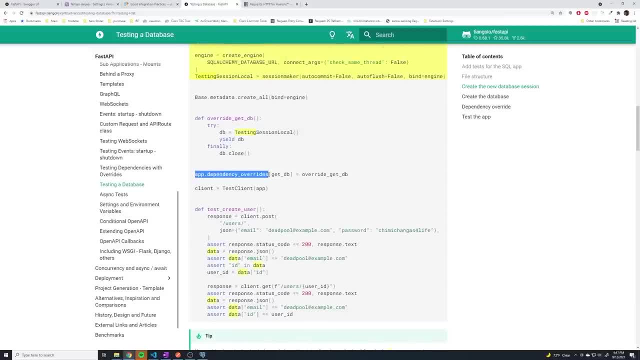 And to override it. Okay, So to override it, we just do app dot dependency overrides. we pass in: well, we specify the dependency we want to override, which is anything with get DB, and then we want to override it with override underscore get DB. 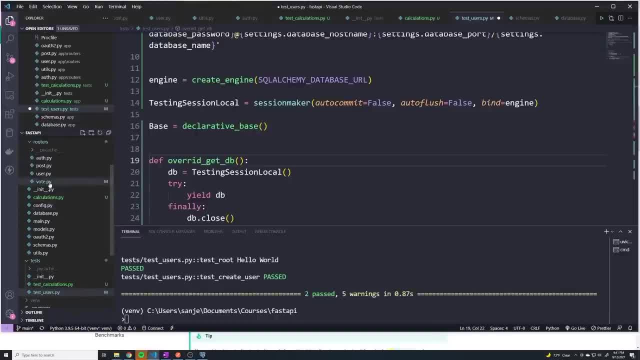 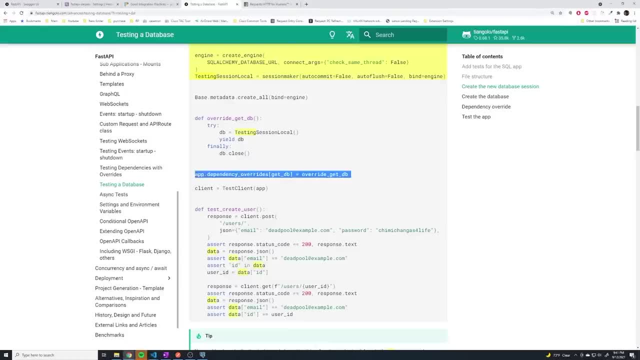 So essentially all that's really doing is in the functions any of our routes right. you can see we've got this. depends: get DB. So when we run that command right here, this override, all it's going to do is it's going. 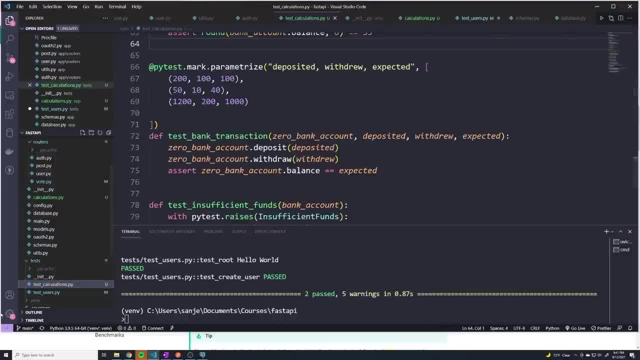 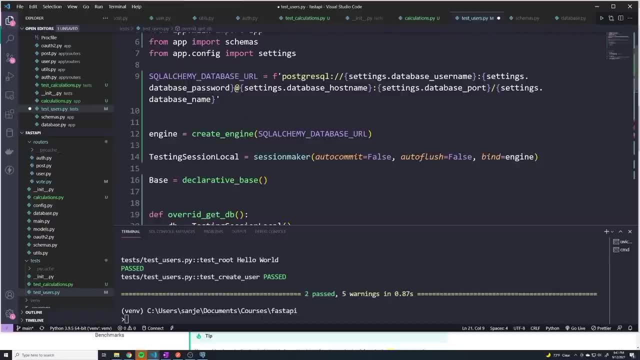 to swap this out with the function that we have right here under test users called override get DB, And it's going to give a different session object And this session object can point to another Postgres database. That's all we're doing. 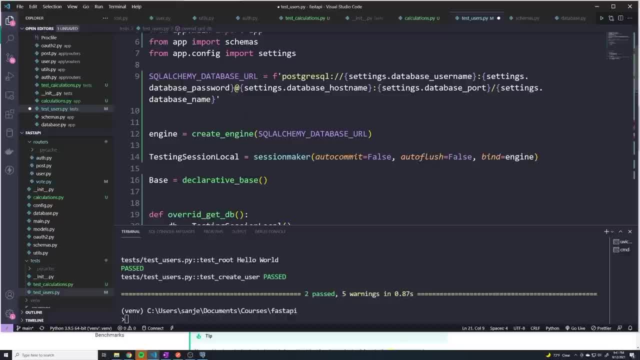 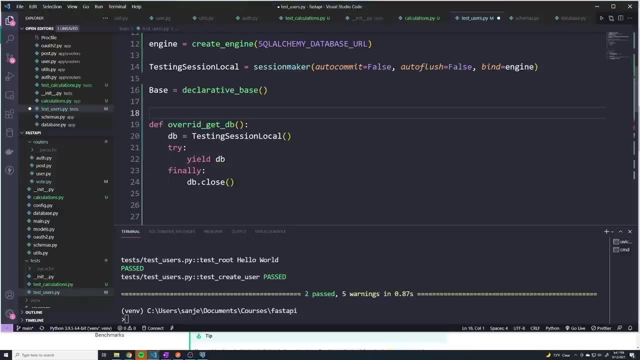 It's really that simple. That's why we set up that, that dependency, when we first started configuring our database, so that we can easily test this during testing, because we can just use the override functionality that's used within a fast API. So I'm going to copy this: 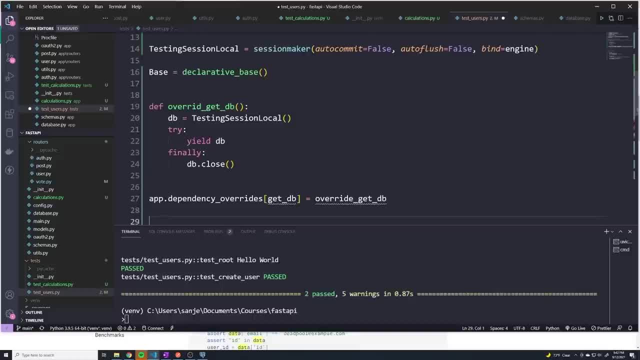 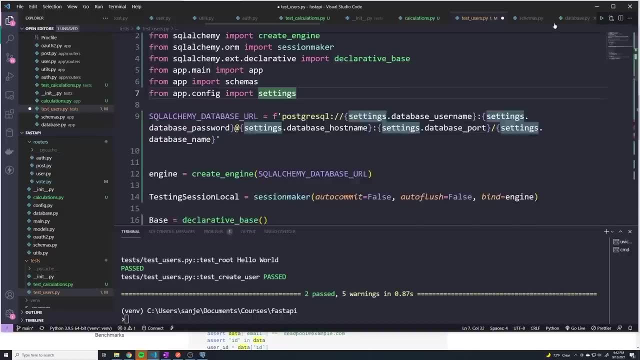 And right here I'm going to paste it down here- And I realized this. I just misspelled override. But we do have to import, get DB now, So let's import that. they'll say from app database: import, get underscore DB. 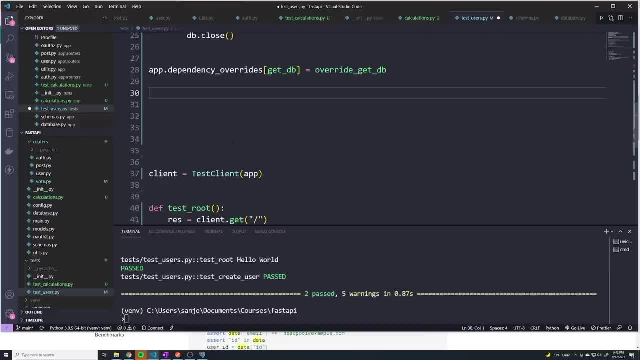 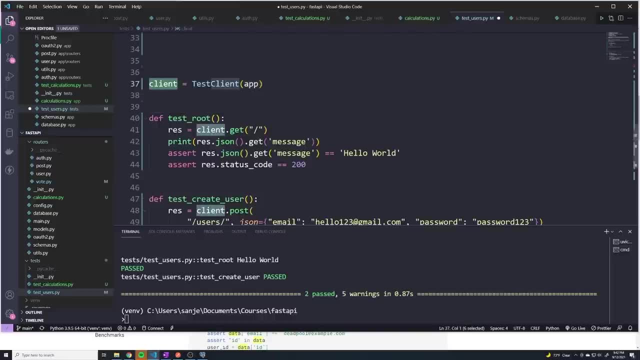 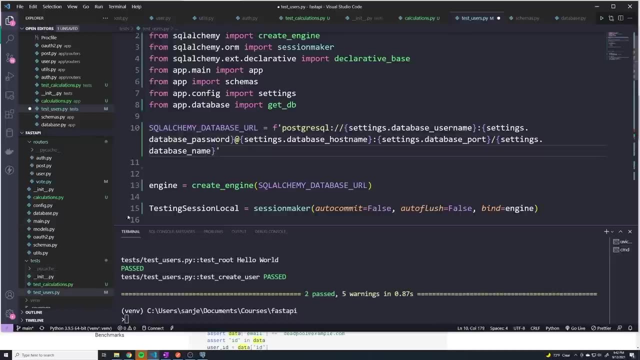 And so it's going to swap the dependencies out, And since we're still referencing the app object, we're going to pass it into test client, And so now, anytime we use this client, it's going to use the new database. Now, currently, our database is using the environment variables, which, once again, is going to put 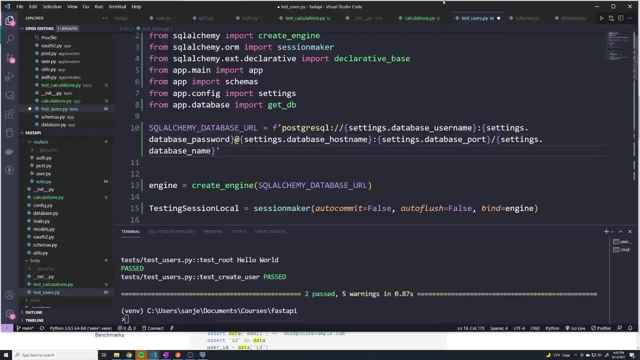 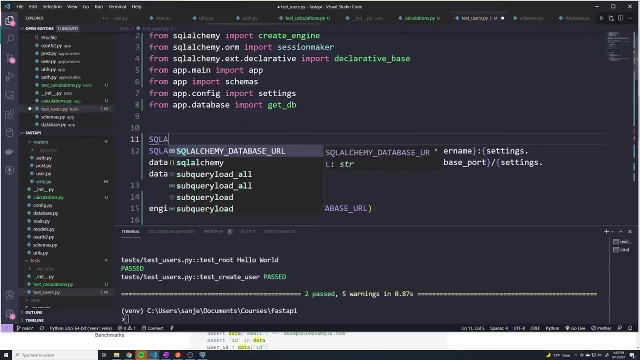 into our development database. So there's a couple of things we can do. Since this is testing, we 100% could just hard code our URL because I mean it's our testing database. who cares if our password and our information is already out there? 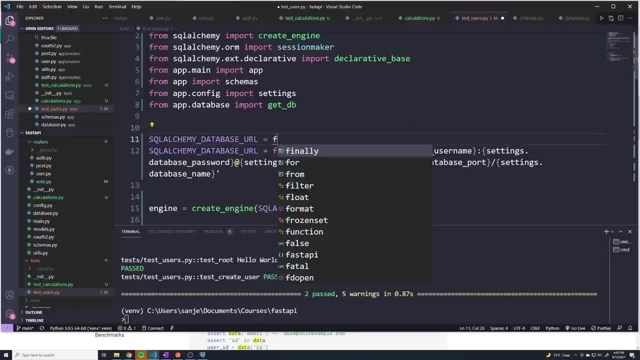 So we could technically do an F string. Actually, we don't even need an F string, I could just say: Postgresql- whoops, there should be a string. Postgresql colon, slash, slash, the. then we have this, And then we have a string. 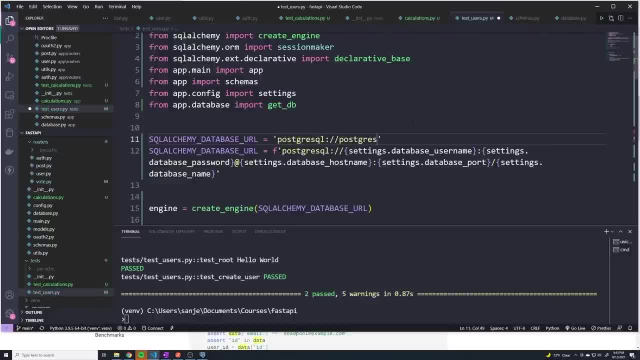 And then we have a string, And then we have a string, And then we have the username- Right now for my, for my database, it's just Postgresql- And then we have the password, which is password 123.. Remember, this would technically be for your testing database. 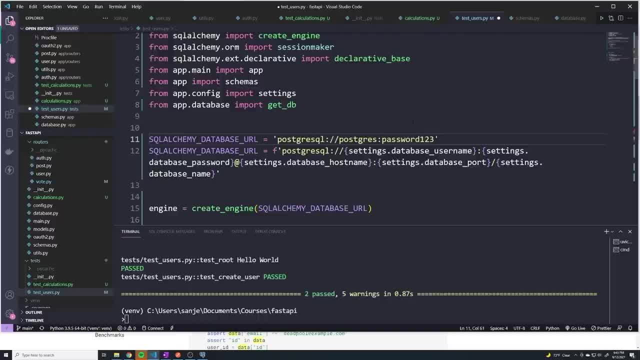 So it's not technically a problem if you put this in there and hard code it. However, you'll see that we could just use the environment variables and make a small tweak, But I'm just going to quickly write this out for you guys, if you wanted to see it. 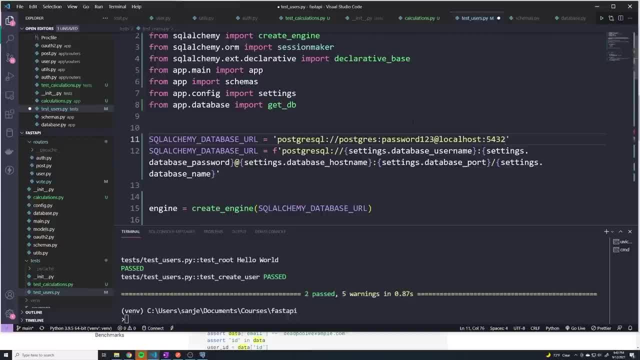 And then the host name is gonna be localhost Ports can be 545.. Okay, And then our database name. so we could call this. you know my print, my development database, is called fast API. I could call my testing database, maybe fast API underscore test. 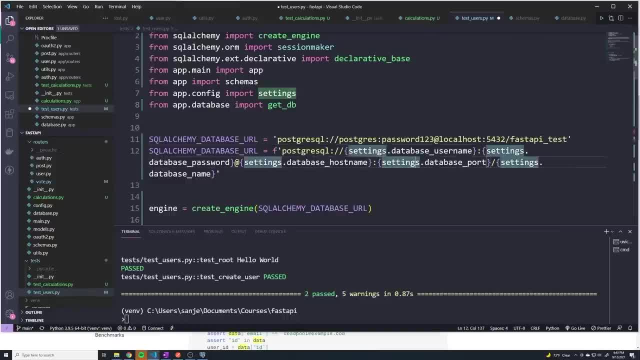 So whatever my project name is, and then underscore test, you can call it whatever you want, And so I could just hard code that and then comment this out, Something like that. Or I could use this same thing but just do a underscore test here. 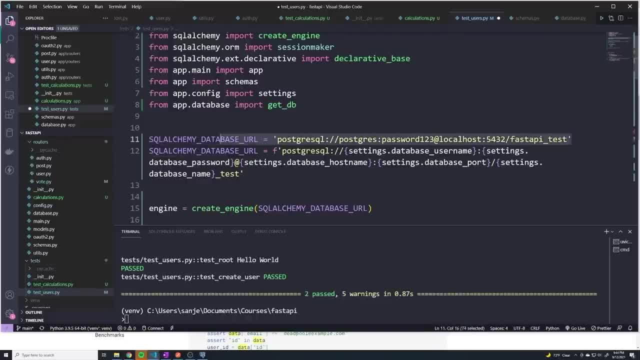 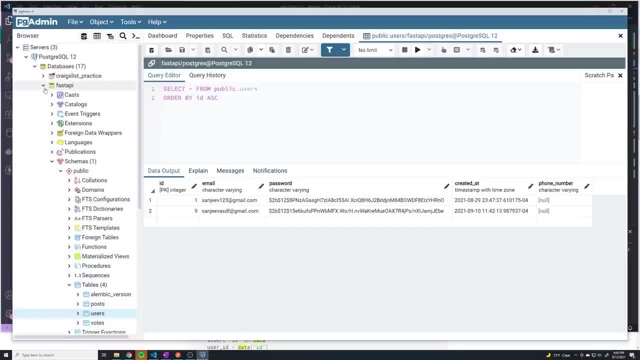 And so that way I don't have to hard code anything. it's going to actually pull it from the environment variables. So whichever method works for you, ultimately that's all that matters. Now I technically already have a fast API test database. 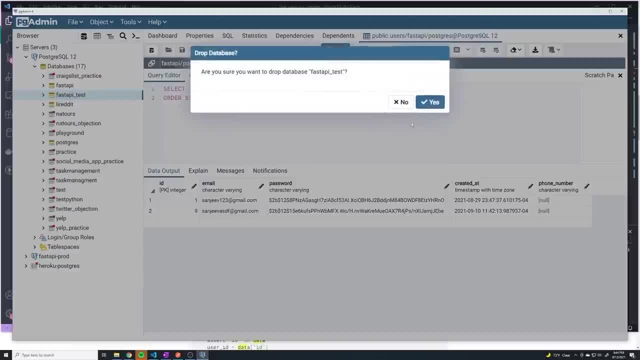 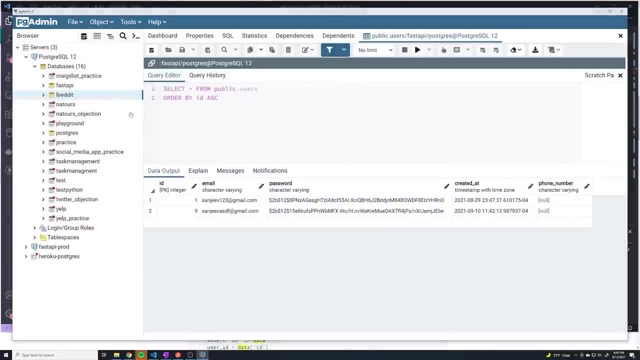 So I'm going to actually delete this. for now, we'll say delete, drop. Alright. so I'm now in. however, your Postgres instance is set up, But since we're going to be using a database called fast API underscore test, we actually 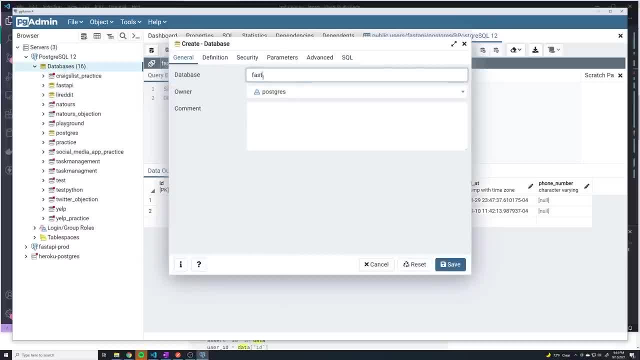 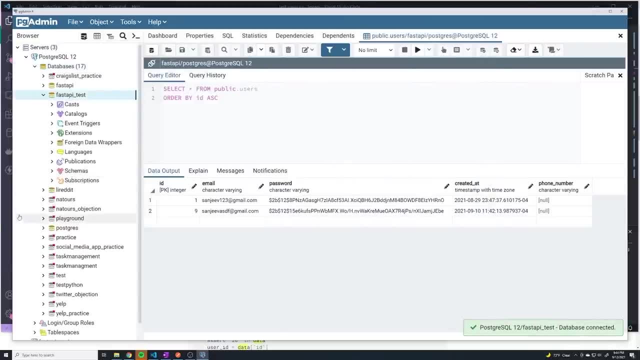 have to create one. So I'll say create database And I'll say: fast, API underscore test. Okay, Cool, Okay. so we've got our test database created And we've set up the override. Let's now actually test this out. 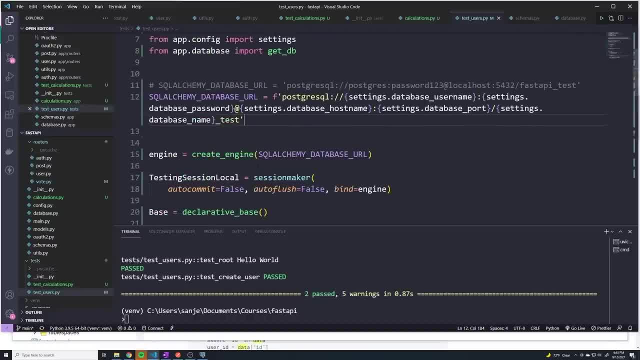 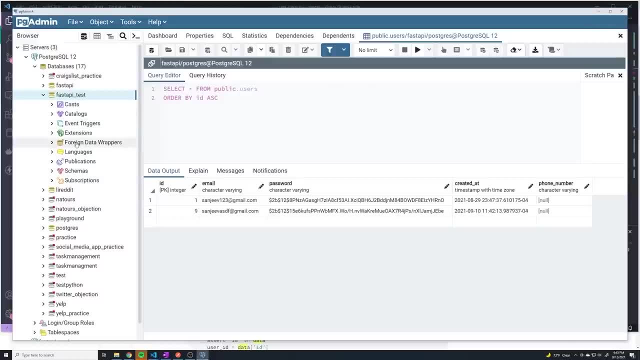 So we're going to do one last thing And I realized, since we have a brand new database, there's no tables, right? If I go down to schemas- tables- right, there's nothing there. So we actually have to build out our, our tables. 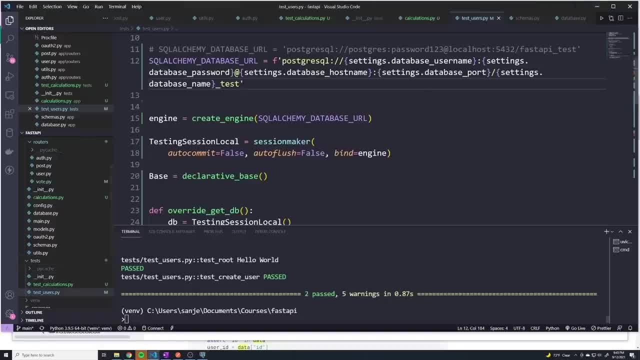 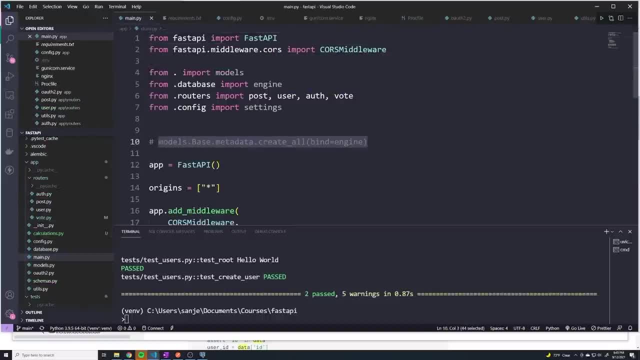 Okay, Before we actually do anything. So easiest way to do that is just copy where's my main file. here we go this command right here. So this will tell SQL alchemy to build all the tables based off of the models we could. 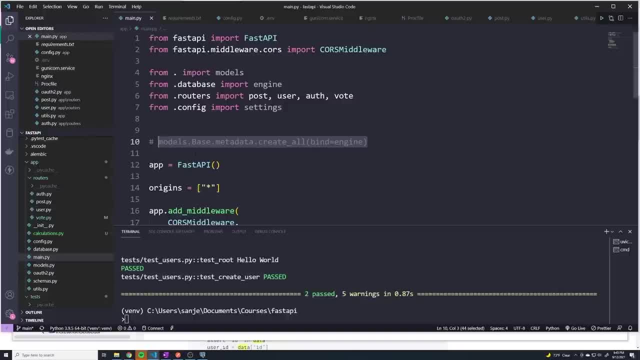 use alembic as well. So I'll show you guys how we can kind of get alembic set up in our testing database so that it actually performs the migrations before test. But for now we're going to keep things simple And we're going to use this. 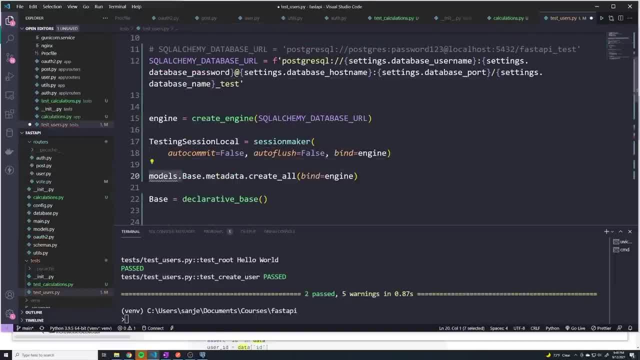 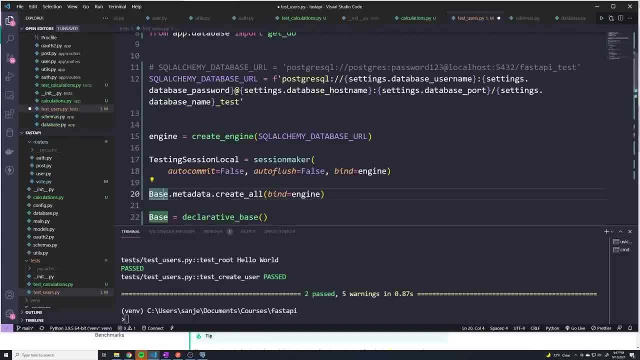 And so I'll just paste it right there And we can remove this models. I don't know why that's there, And you can see that we get a warning right here So we don't have anything based, So we actually have to import that from our database file. 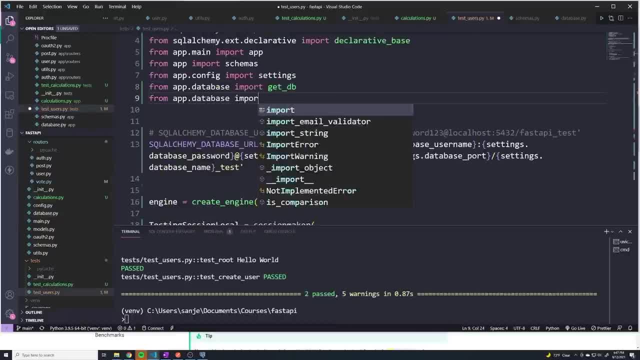 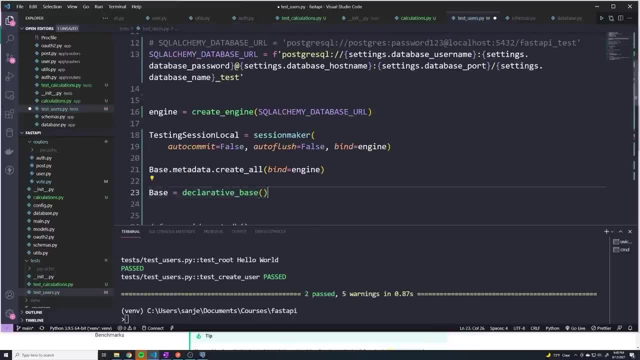 So I'll say from app database import base, And I realized we actually don't need this line right here, So we'll remove that. All right. so now our test database is completely set up And when we, when we add our test database, we're going to get our test database. 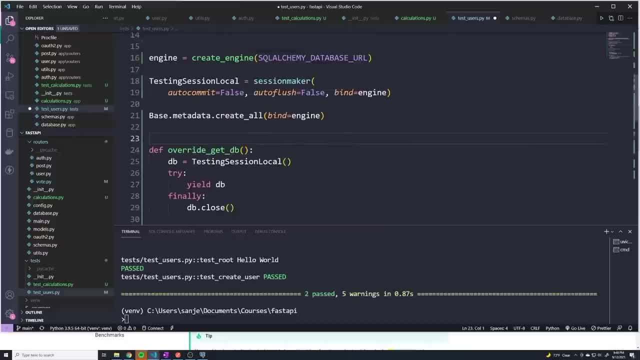 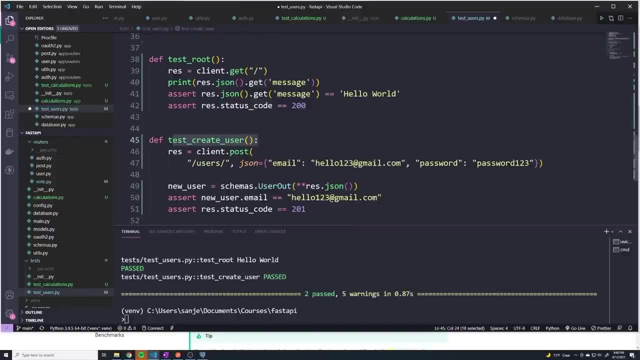 And when we, when we add our test database, we're going to get our test database, And when we, when we actually run our first test, it's going to run this right here, which should create all of our tables for us. So let's take a look at our test: create user. everything should be good. we shouldn't have. 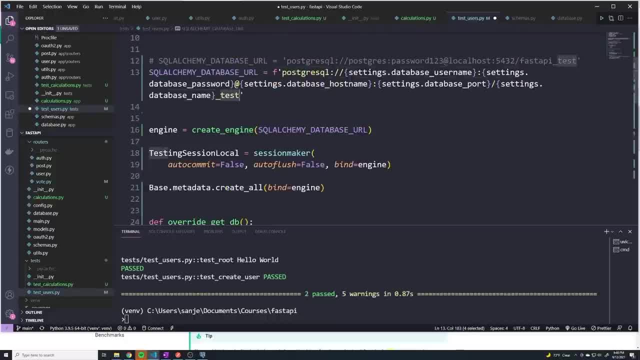 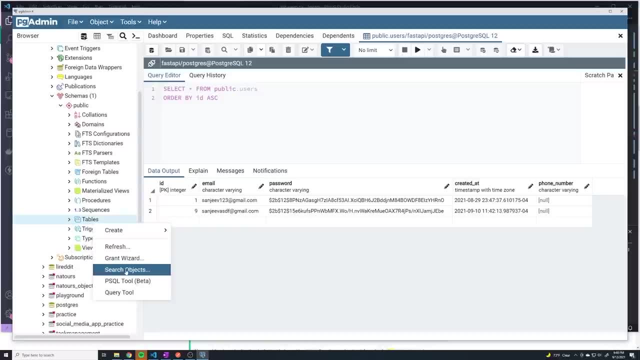 to touch anything And our URL should point to fast API underscore test. So let's try this out And I'm just going to refresh this And yep, we shouldn't have any tables. Good, Perfect, And let's run this now. 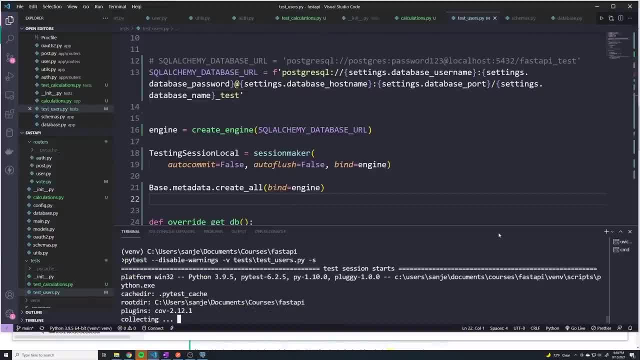 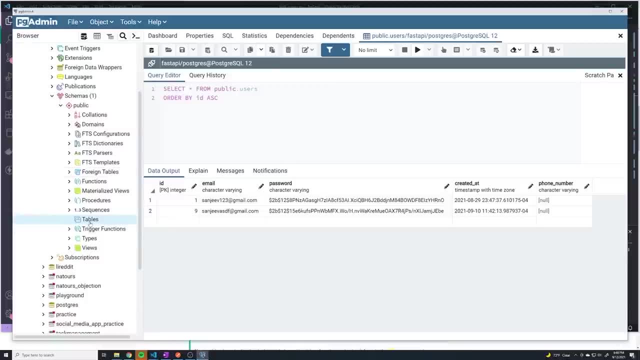 So let's run just the test users. All right, and both of them passed. So how can we verify both of them past? Well, let's go to our tables. I'm going to refresh this. we can now see. we've got all. 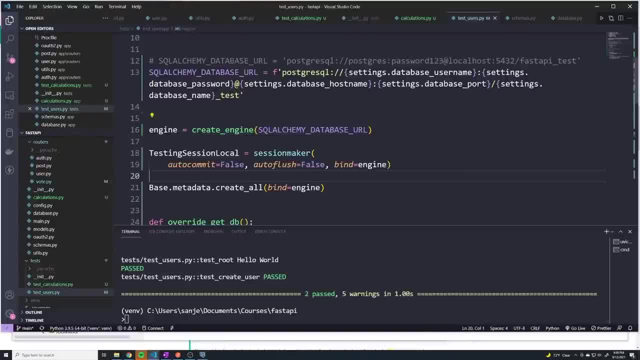 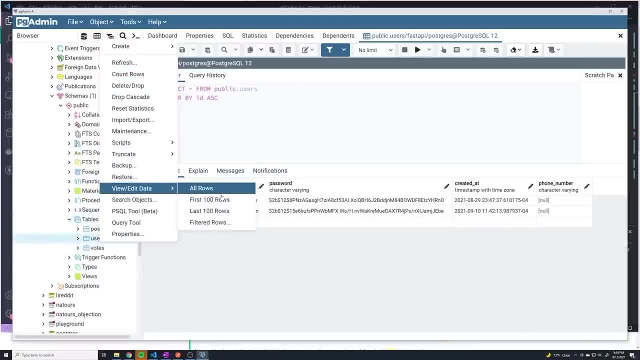 three tables right, And that's because we ran this specific well, not that command, this command right here. And if I do a users, and then where is it? if you edit a, all data, all rows, right? we? 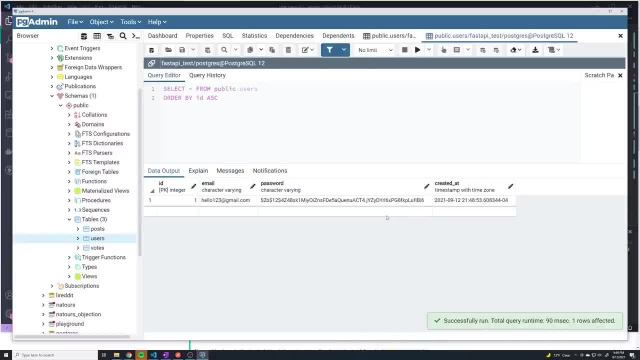 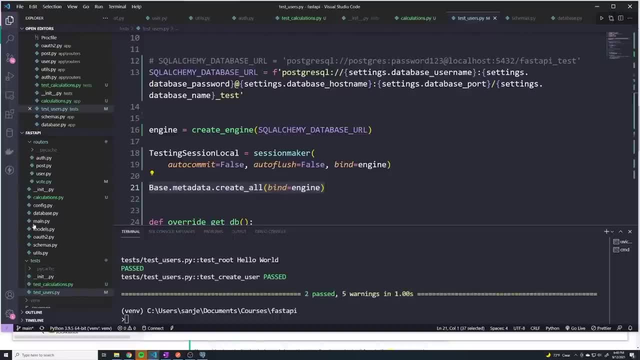 can see that our user was successfully created. So now we have now gotten our test database. So now we have our test database set up so that we no longer interfere with our development database And keep in mind: right, it does. your test database doesn't even have to run on your. 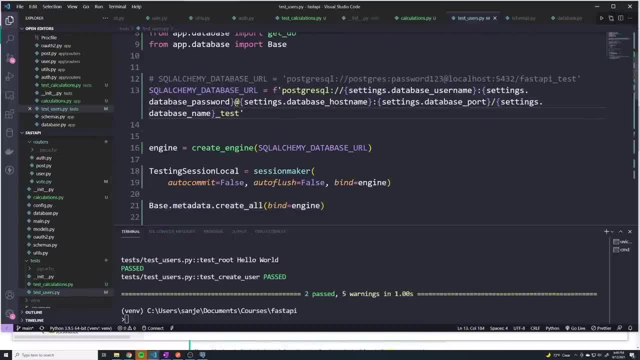 local machine. you can run it anywhere. you can run it in a Docker container, you can run it on a remote machine. you pass in the details of your test database and then your testing environment will handle the rest. So, now that we've got our test database and we've successfully ran our tests- if we run- 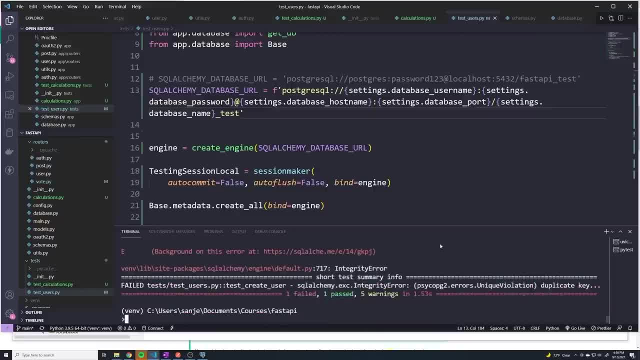 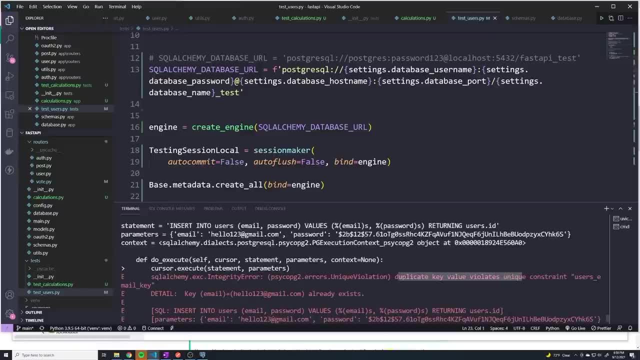 our tests one more time. take a look at what happens. we get an error right and we get an error Now. before in our development database we already have a user, So we get this. duplicate key violates unique constraint because this user already exists. 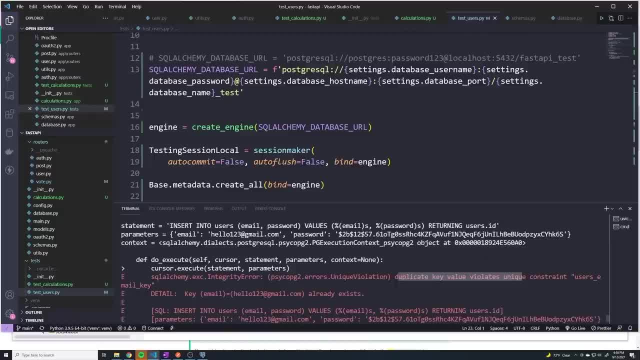 So when we run this again, we try to create a new user with the same exact email, And this obviously causes things to break. And so how do we get around this limitation? right, I want to be able to run my tests as. 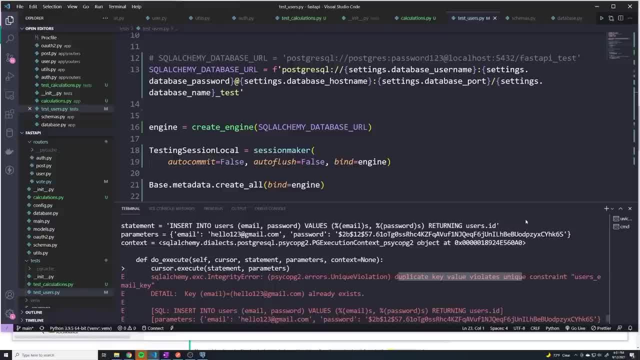 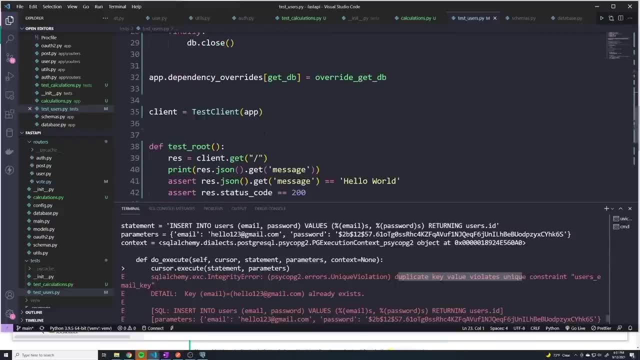 many times as possible, And I wanted to kind of start out with a clean slate. Well, we can make use of fixtures. So let's take a look at our fixture, And if you already forgot what a fixture was, it's just a function that runs before your. 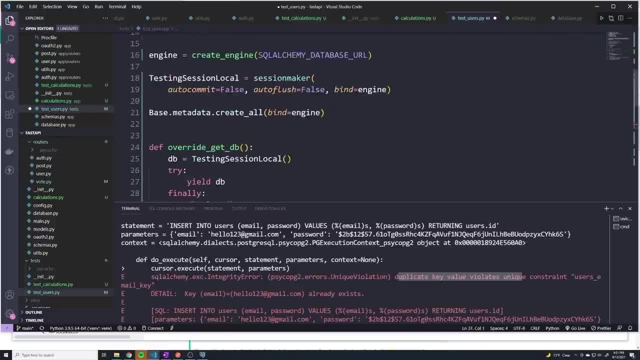 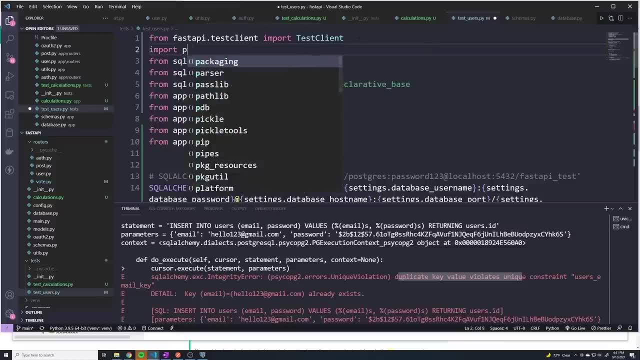 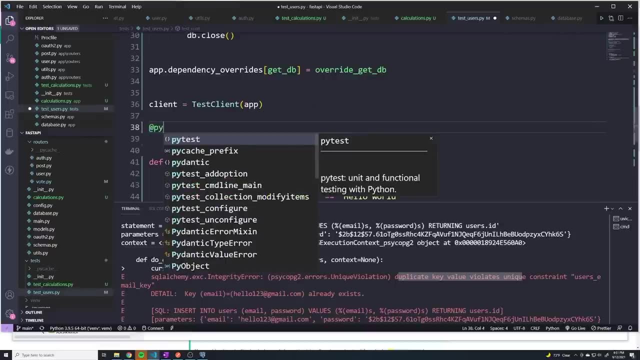 test runs. I'm going to create a fixture And I'm going to have to do: we already import pi test. we did not import pi test, So let me import that in here. We'll say: import pi test And I'm going to say: I'm going to create my fixture. 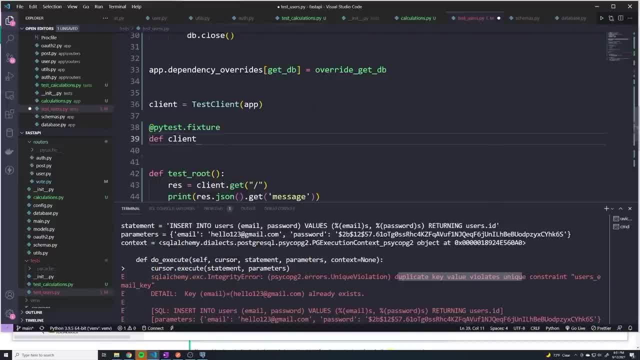 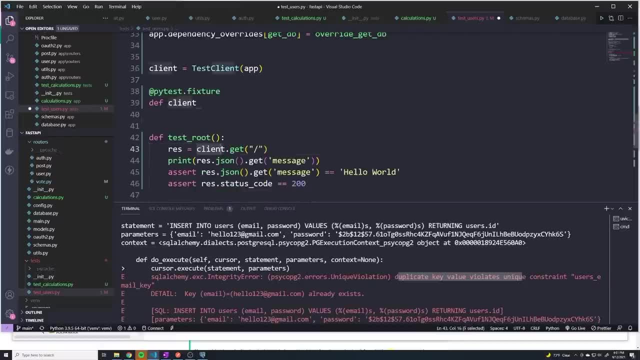 Call this whatever you want. I'm going to call this client. So this is actually going to return. is actually going to return our client Right? This is our client object right here, which is the test client, which is what we use to. 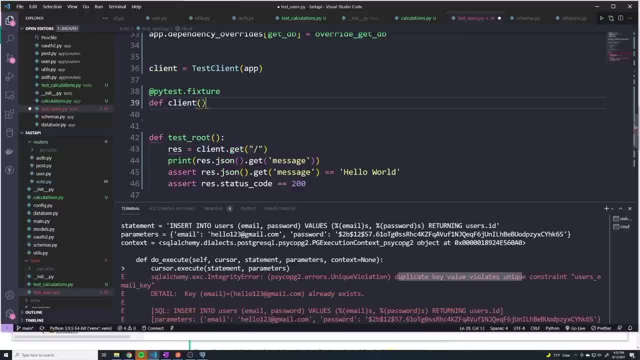 actually generate the request. So I'm going to call this def client And what this is going to do is I'm going to remove this line right here and just copy this And I'm going to say: return this And we can just remove this line at that point. 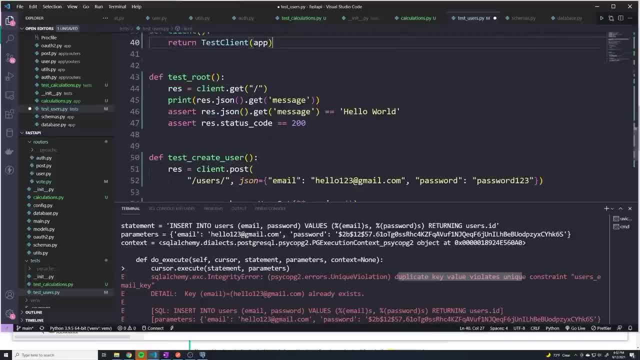 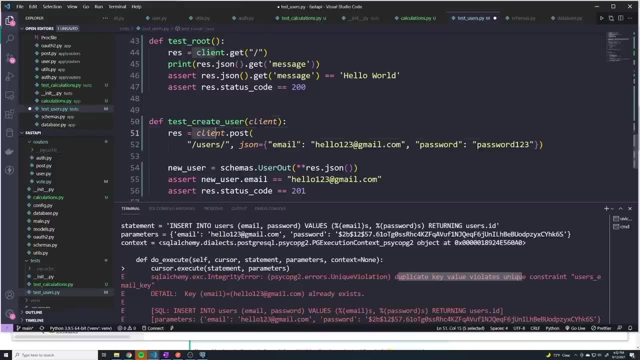 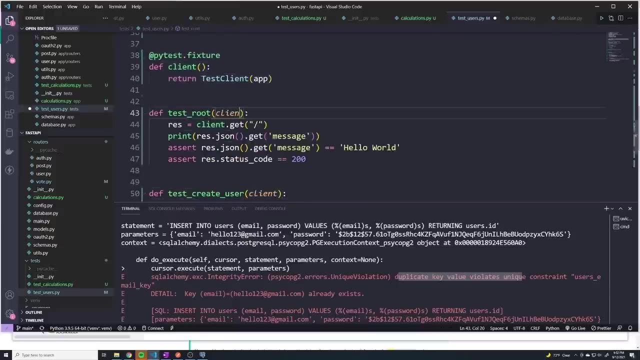 So this is going to return our test client instance, And so now, to get this to actually work, I'm going to pass in our client, And so now this client object references the client that we get from this fixture, And we'll do the same thing here. 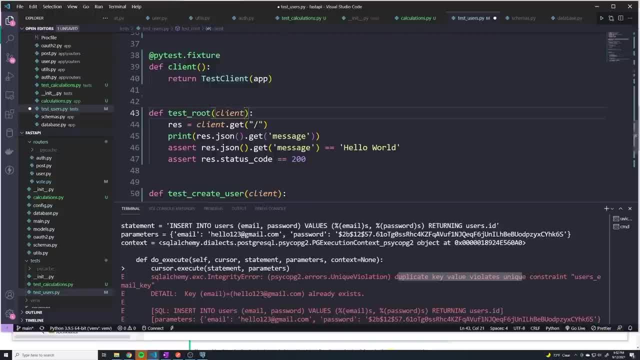 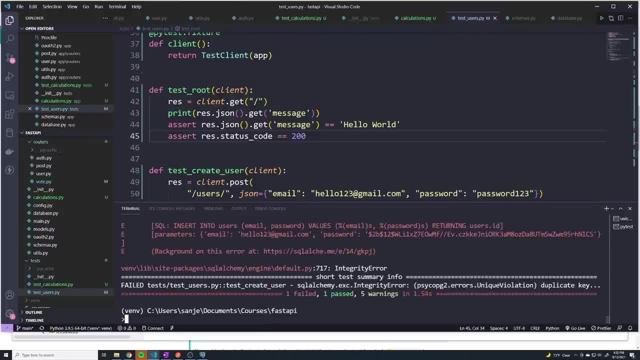 So what exactly has this solved? Right now, it hasn't really done anything for us, right? our code is going to work exactly the same. You know, if I save things and run it again, right, same exact issue, and obviously I can. 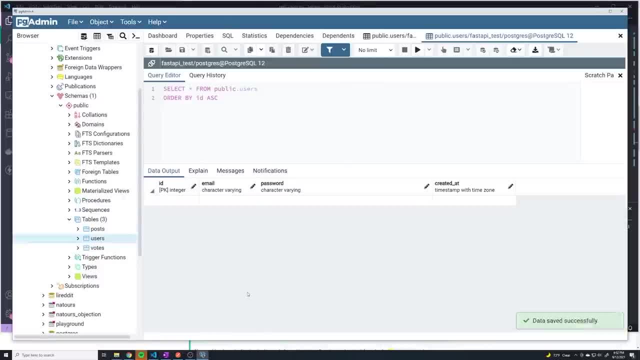 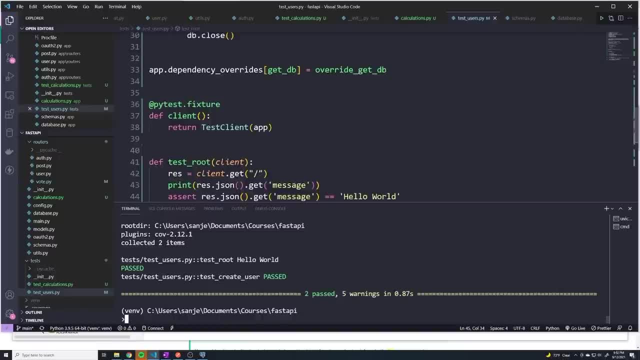 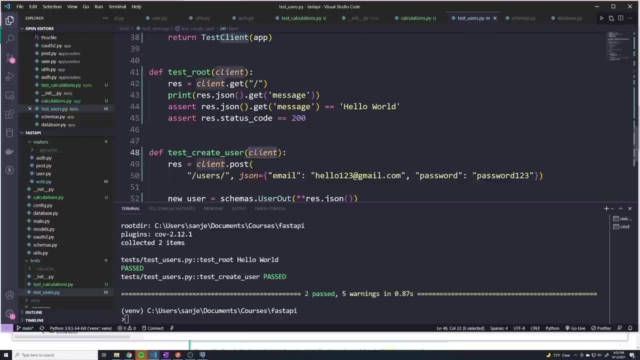 go in and I can delete this And then run this. Right, it's going to work just fine. But it is nice because we now have this function that runs before each one of these tests. that gives us our testing client. And what's even better is I can actually change this a little bit. 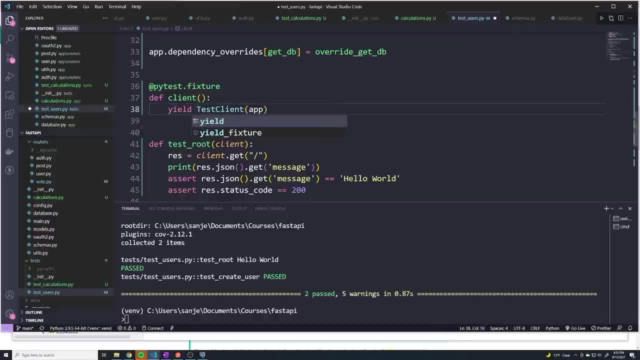 Because I can change this to be a yield right. when you change it to yield, what it does is. it gives us a little bit more flexibility because now we can, you know, run our code before we run it, So we can return our test client. 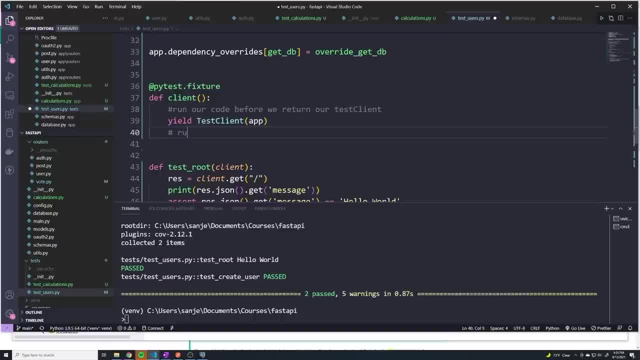 And after the yield we can then run our code. actually, this should be run our code before we run our test, and then this is going to run our code after our test finishes. So now we can put in logic, for you know, what should we run before our code runs or before? 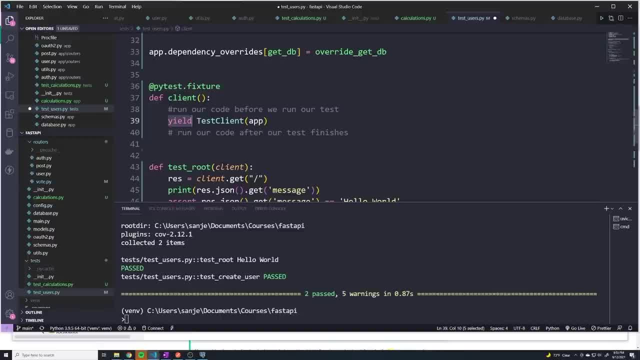 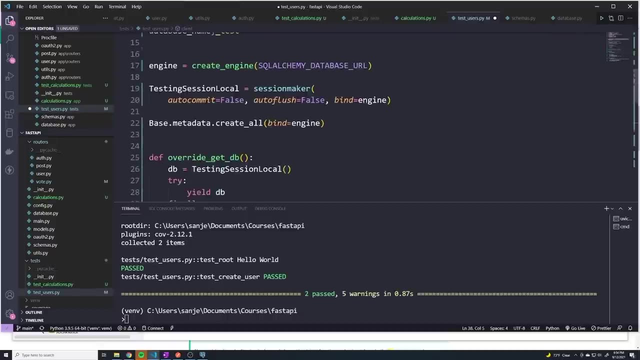 our test runs. we then yield, which is the same thing as return. it's going to return our test client, And then we can run some code after the test finishes. So what we can do is before our code runs. I can copy this line right here: 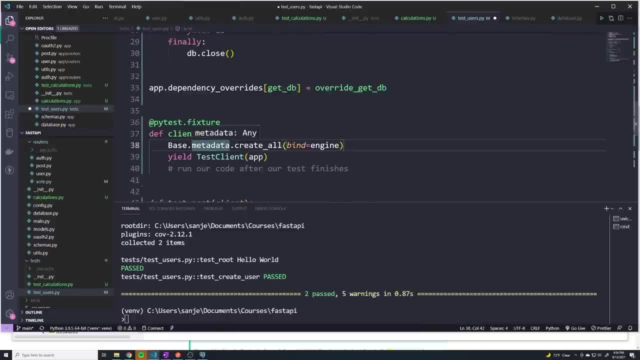 So, before our code runs, I can create my tables And then, after my code runs, I can drop my tables. If you want to drop a table, you just run base dot- metadata, dot. drop all instead of create instead of create all, and it's going to drop these tables. 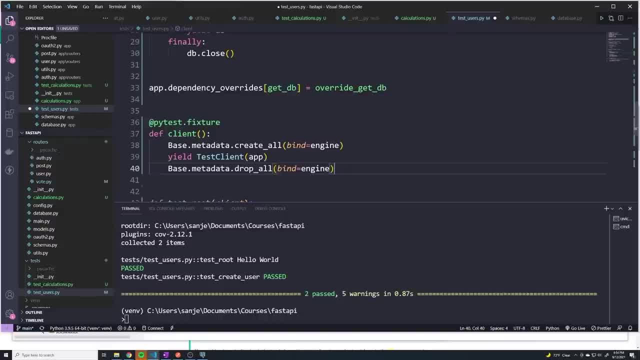 And so now, every single time my tests run, I'm essentially going to be starting out with the clean slate. it's going to drop all of our tables, all the data in each table. it's going to return the test client. we're going to run the test and then- sorry it's I messed. 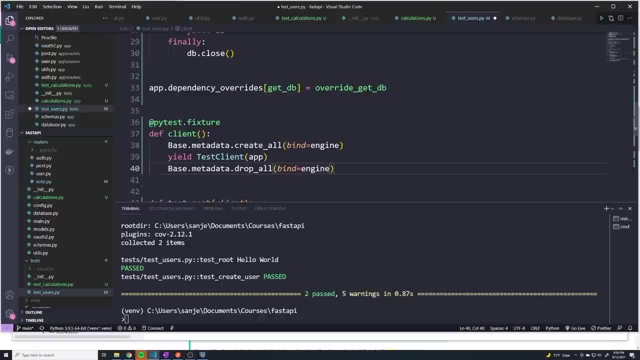 that up. So when we, when we finish a test, we're going to drop all of our tables, delete our data. then the next time the test runs, what's going to happen is we're going to create all the tables again, because there's no tables. we're then going to run the test. 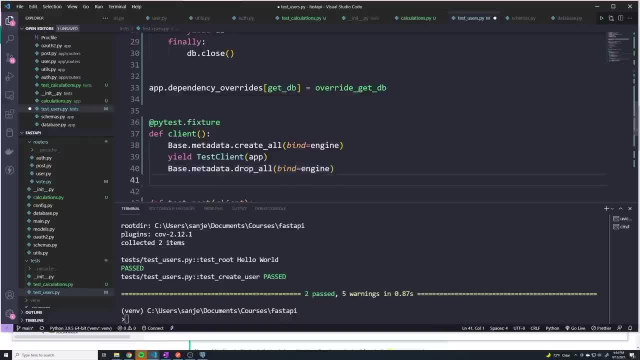 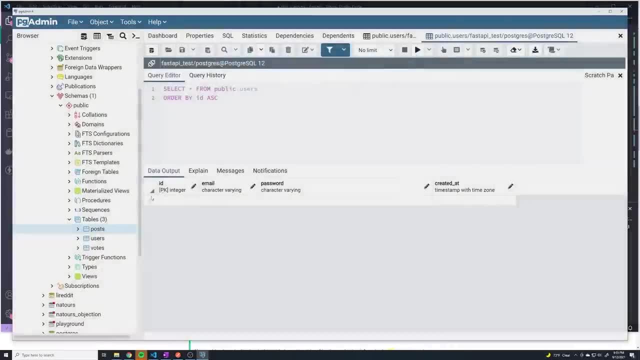 And then, just like we did before, We're going to then drop all of our tables again. So what I'm going to do is, first of all, I'm going to manually drop these And I'm going to have to drop votes first, or that's gonna throw some foreign key errors. 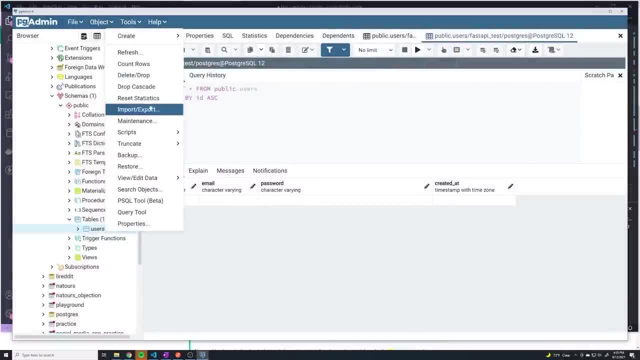 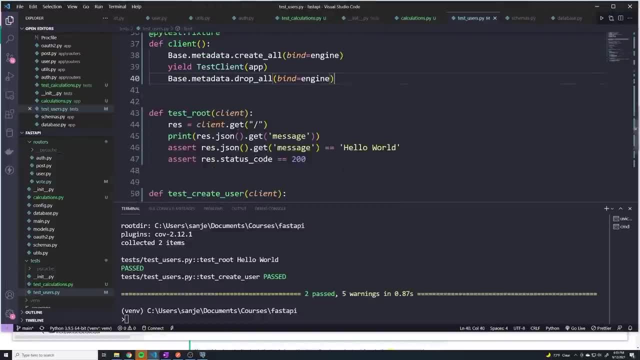 And then we'll drop posts And then users. Okay, so now everything should work, And I'm actually going to test this out. So, once again, just to reiterate: we're going to create our tables, because we don't have any tables. 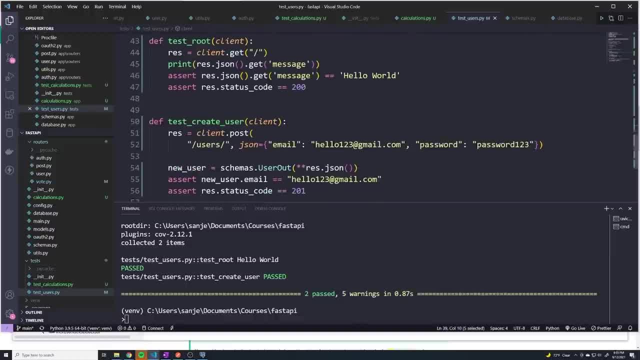 We're going to then run our test. right yield just returns our test client to our create user, and then we can, you know, perform all of this logic. After that's done, we'll then drop the tables again, So we start from scratch the next time around. 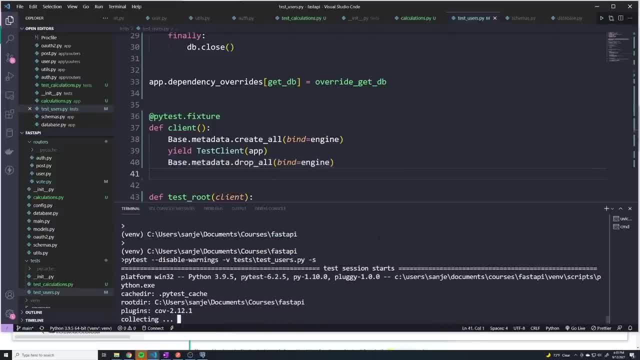 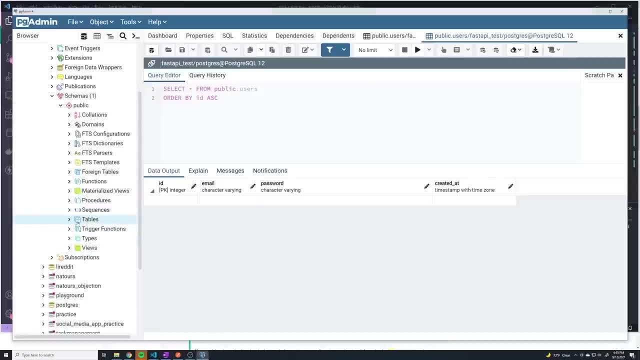 So let's try this out. All right, everything's worked. And if I actually go back to here and hit refresh tables, you can see there's no tables because we dropped the tables after we're done. And if I run this again, it works. 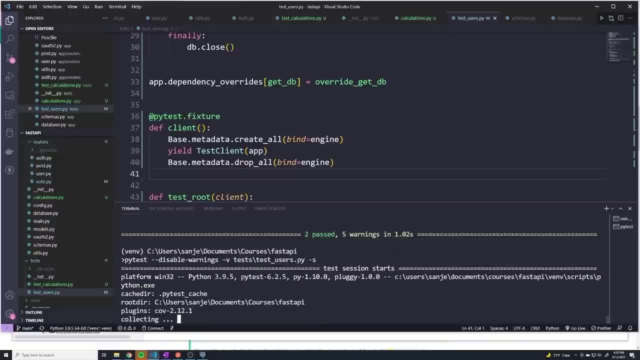 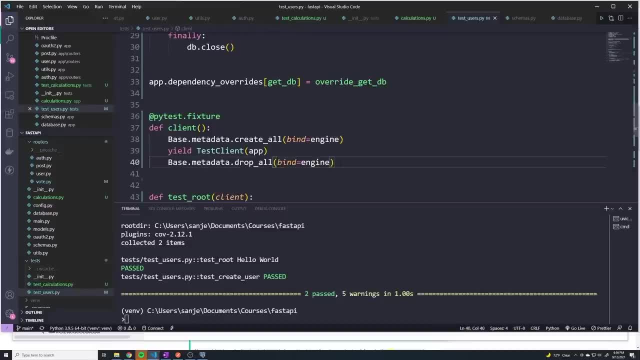 We can run this as many times As we want. We don't have to worry about duplicate users, because we're clearing out our database. And there's one more thing that you can do as well. If you wanted to, we could actually take this drop all and move it up here. 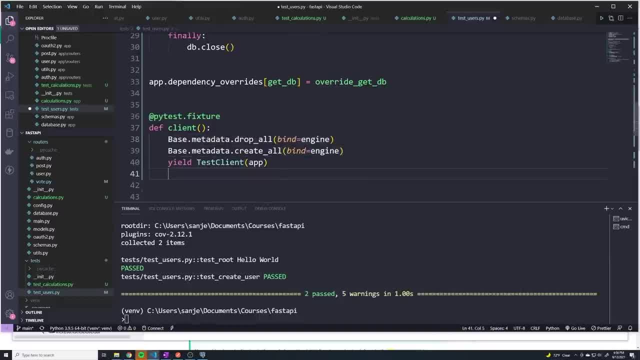 So what's the what's the benefit of doing like this, Or why would you want to do it like this? Well, the nice part about this is right. it's going to clear out anything we had previously. it's going to create our tables and then it's going to run our test. 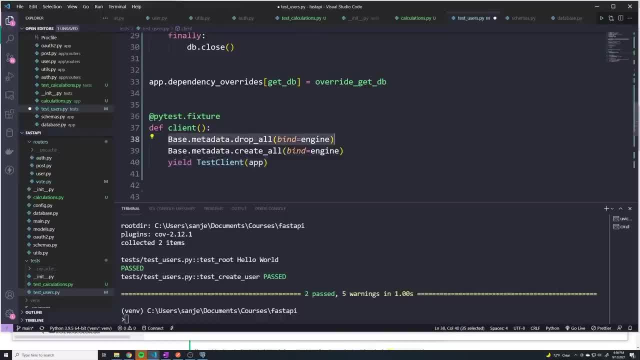 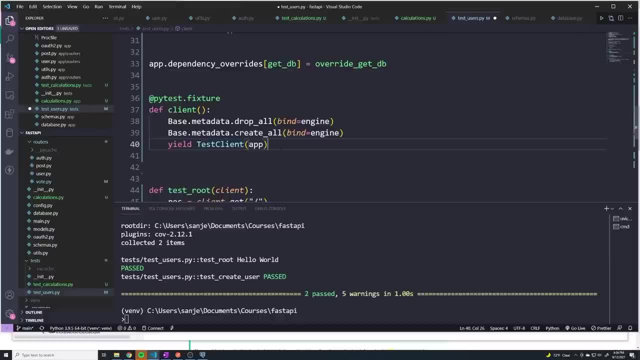 And then the next test that we run, we're once again going to clear out our table. Yeah, we're going to clear it out, and then we're going to build our new tables again. So this way, if you, if your test fails, you can, you know, pass in the dash, you know. 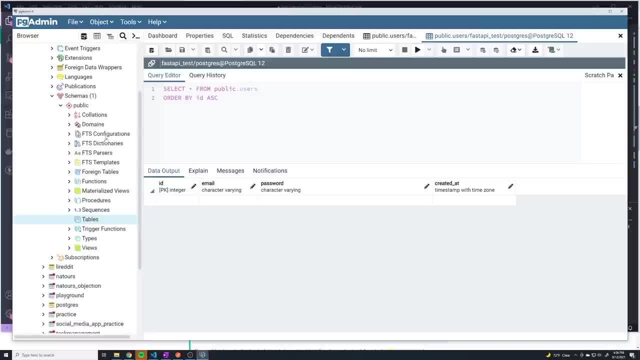 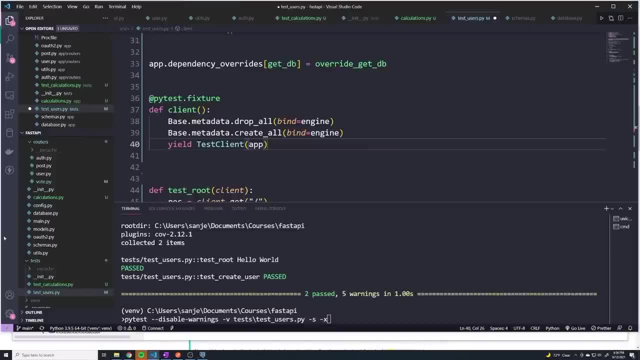 X flag to stop after it fails. And what's going to happen is it's going to keep all your tables and all the data so you can see what was the current state of your database when the test failed, so that you can- you know, ideally have a little bit of better idea of what's happening. troubleshoot: 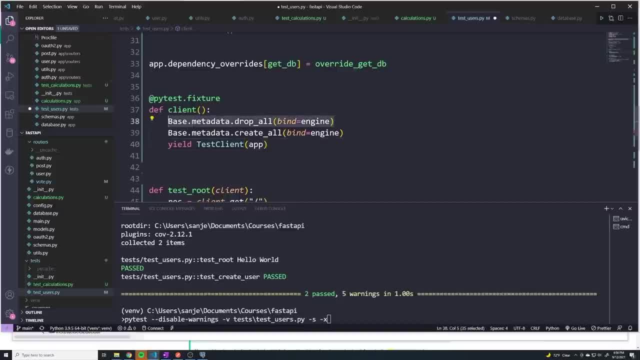 a little bit more, because you have access to your to your tables, Whereas if it's- if this is down here, right, it's just going to delete the tables after you're done, Right? So it's a matter of personal preference, But I like to keep the tables after it's done. 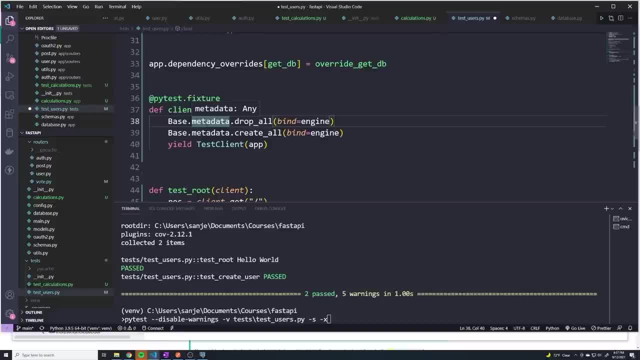 So that you know, if I do want to stop it and just kind of poke around and take a look, then I can. And if you guys don't want to use SQL alchemy, you can do the same thing with Alembic. 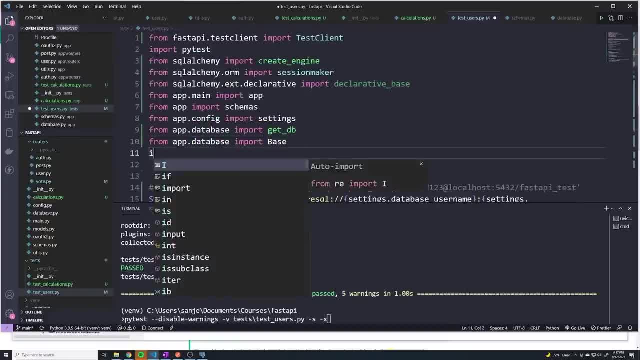 Right, I can, I can import, you know, Alembic dot config. actually it would. I think the technically the import is from Alembic dot config import config. sorry, not that. Nope, nope, It's a from Alembic import command. 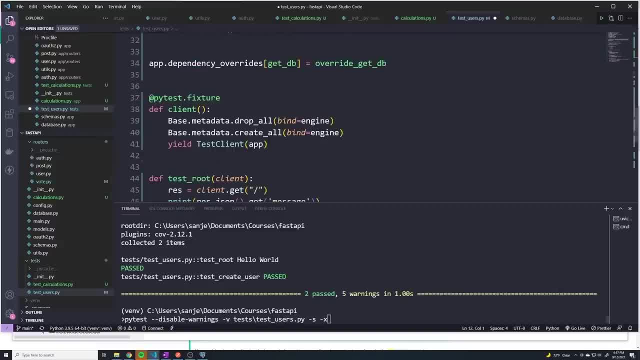 So what we can theoretically do is in here, instead of using these, we could say something like: I think it's command dot, upgrade, so you can upgrade, And then you can go up. upgrade to, I think, head right. 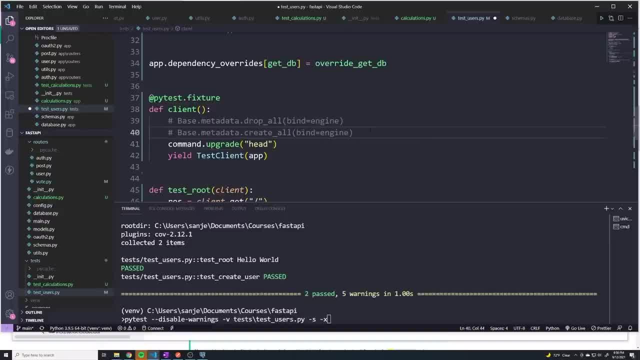 So this will build out all the tables for you And then, after you're done, you could then go in and say command dot, downgrade to base or something right. You'd have to make sure you set up Alembic with all of the right environment variables. 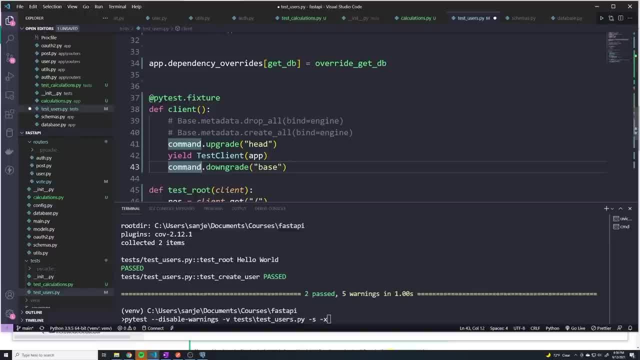 and things like that. But that's all you would have to do if you didn't want to use SQL alchemy's built in functionality. So I'm going to just delete that, just to keep things simple. Now we're gonna let SQL alchemy build the tables for us moving forward, just because. 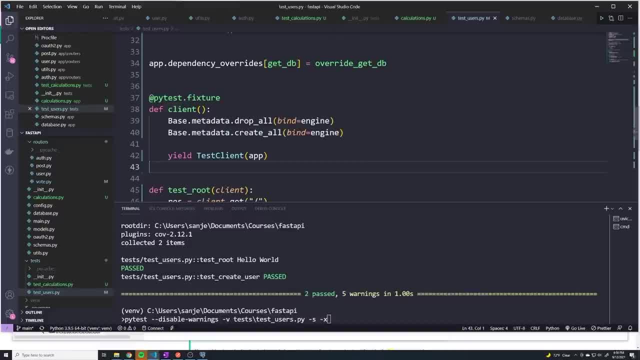 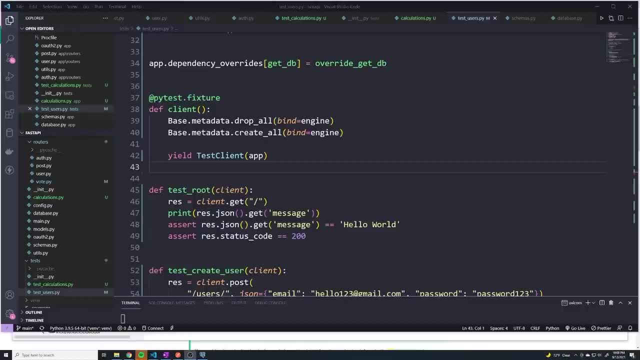 it's a little bit quicker than having to, you know, build all of your revisions and things like that. So one of the cool things with fixtures is that we can actually configure a fixture to be dependent on another fixture, So we can essentially 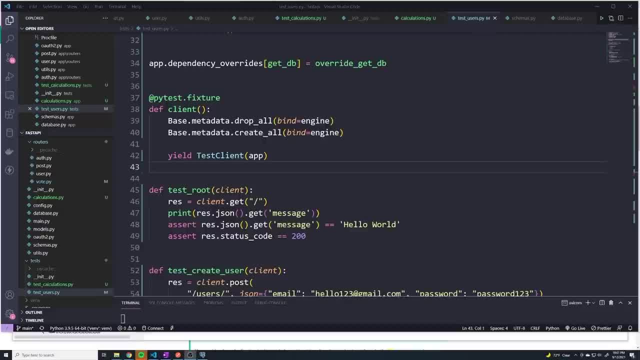 Pass one fixture into an argument of another fixture, And the reason why I want to do this is I want to have one fixture that returns my database object, So if I want to ever manipulate data directly, and I want another fixture that returns my client. 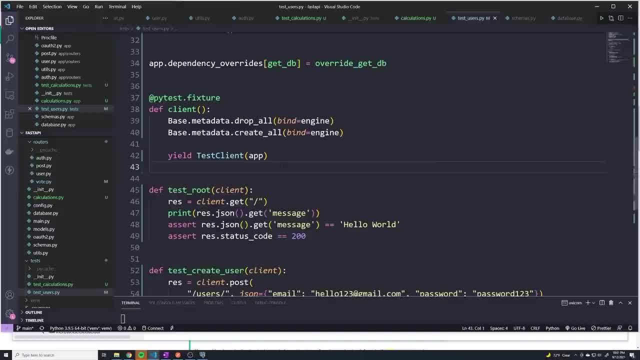 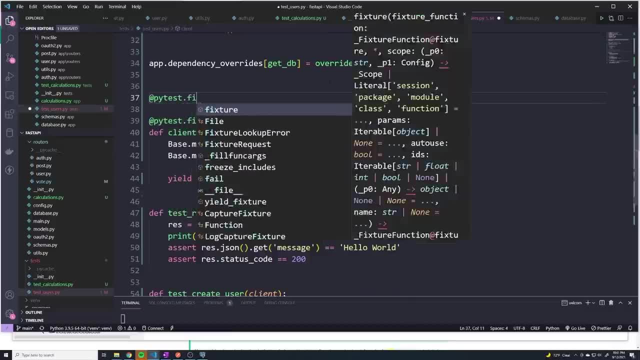 So this, this one is returning our client, So I want that, but I also want another one that returns just our database object. So what I'm going to do is I'm actually going to create a new fixture. I'll say: PI, test out fixture, and we can call this whatever you want. 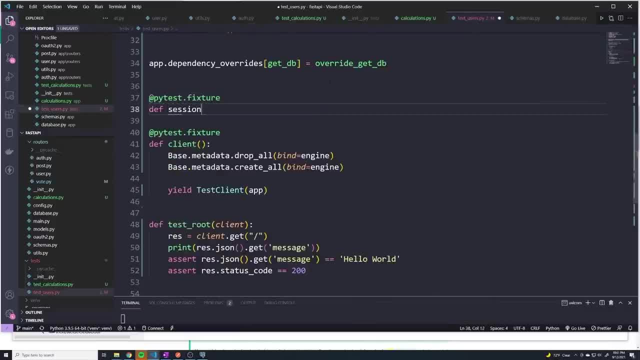 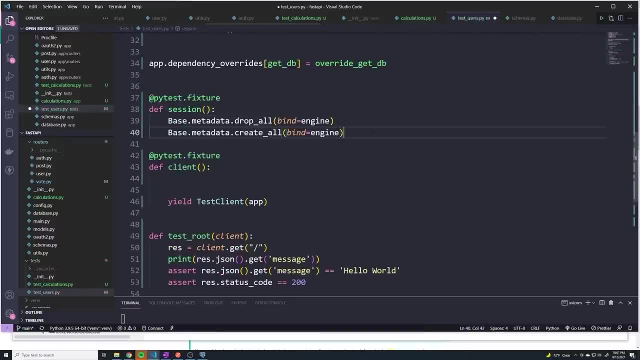 You can call it, you know, like DB or session. I'm just going to call it session, Okay, And I'm actually going to move the logic of deleting and creating our tables up to here, because this is kind of handling all of the logic for the database. 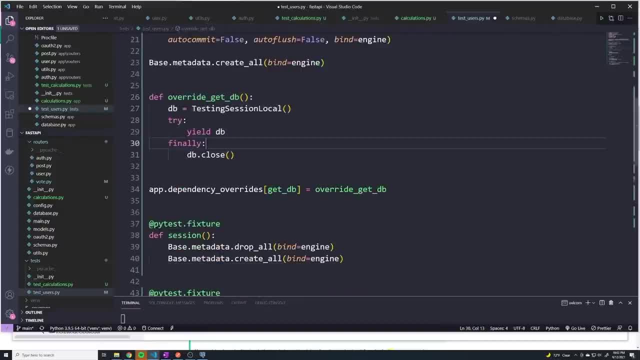 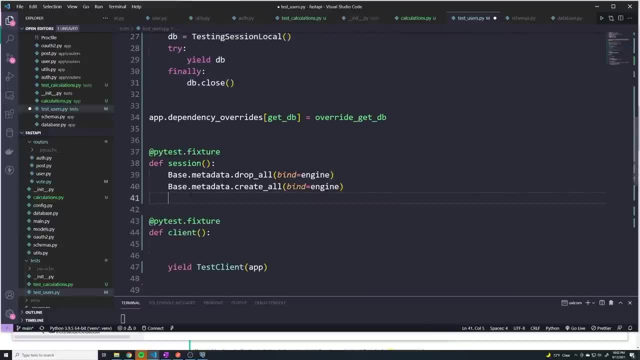 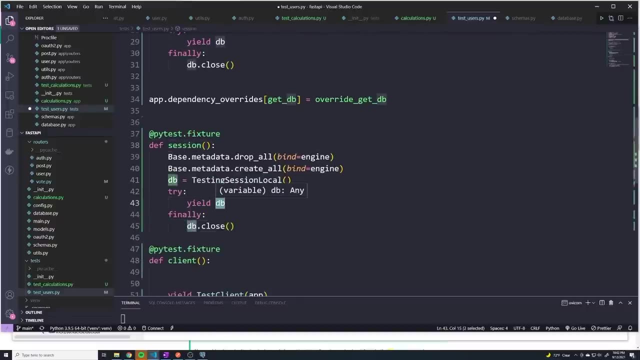 And you see, all of this uh, override functionality. What I'm actually going to do is I'm going to just copy this section right here and paste it into here, right? So this session fixture is going to yield the database object. So the database, the object that we used to query. 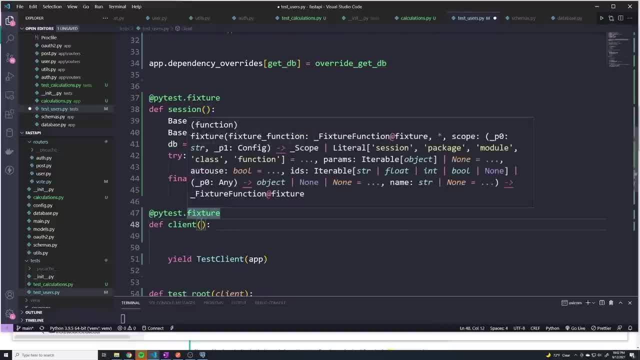 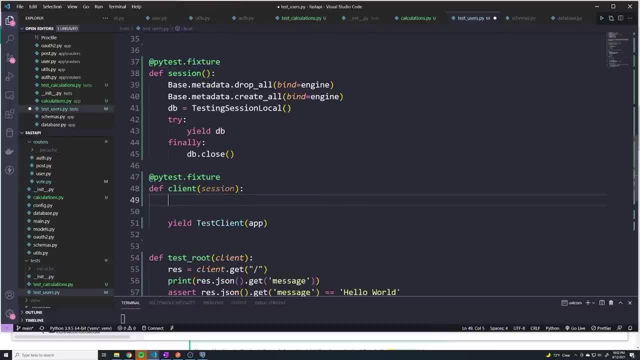 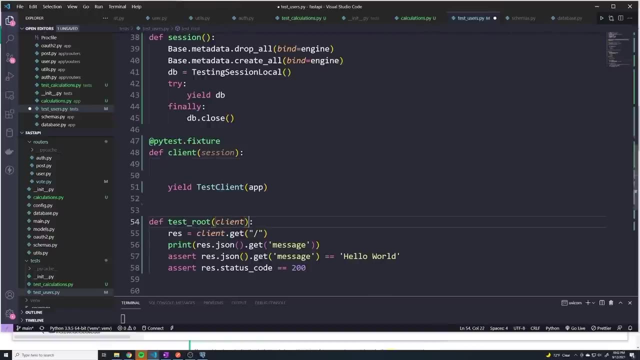 And what I can do now is I can pass in session, the session fixture into my client fixture, And so, by doing it like this, what's going to happen is, any time I go to one of my tests and I pass in the client fixture as a essentially as a dependency, it's going to call this one. 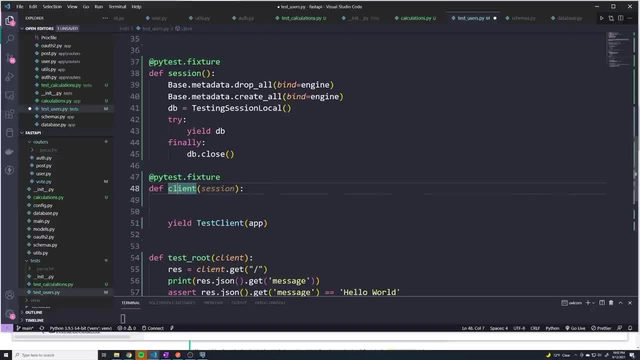 and the client fixture will actually call the session fixture before it runs. So it's intelligent to understand that a requirement for the client fixture is the session fixture. So we're going to run all this code. It's going to return the DB object. 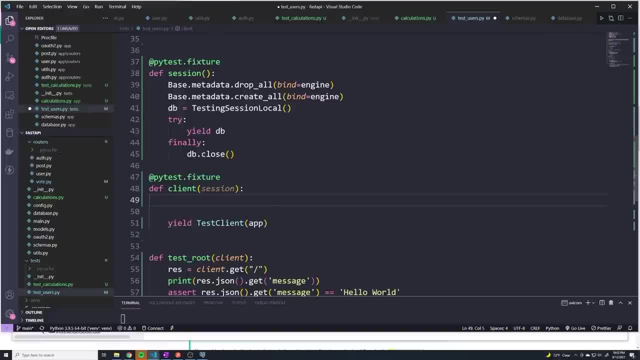 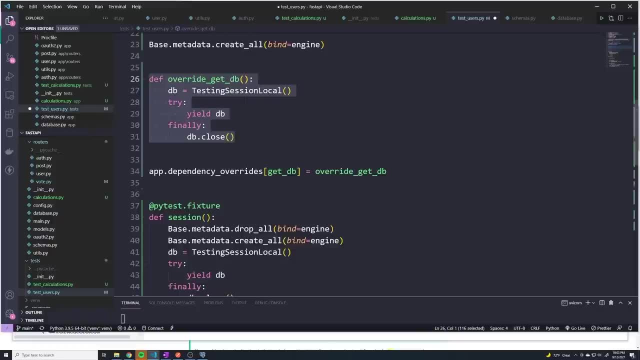 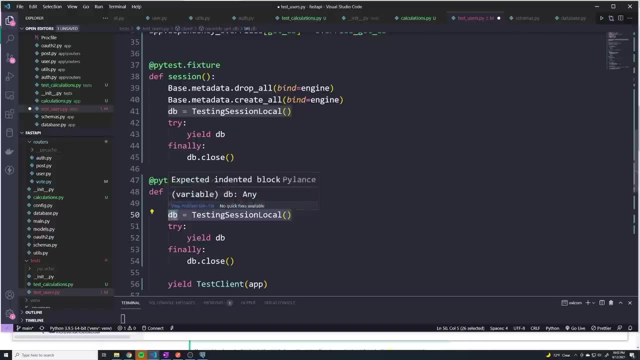 Which is going to be passed into client as the session. And then here we can perform all the logic that we normally would- And I'm going to once again copy this override DB right here And we can remove this And we can remove that. 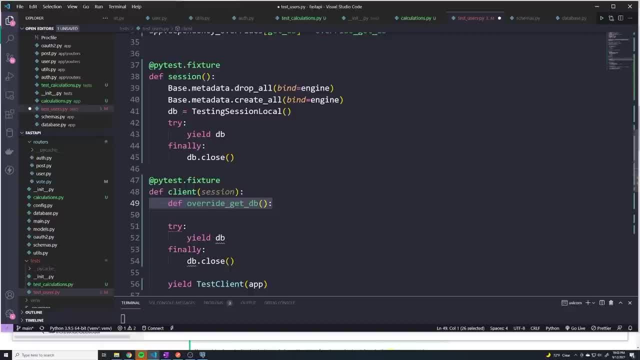 Nope, Actually, sorry, I didn't mean to remove that, Just space these out a little bit. So it's part of the override get DB function And here, instead of yielding DB since there's no DB, we're going to yield session, which. 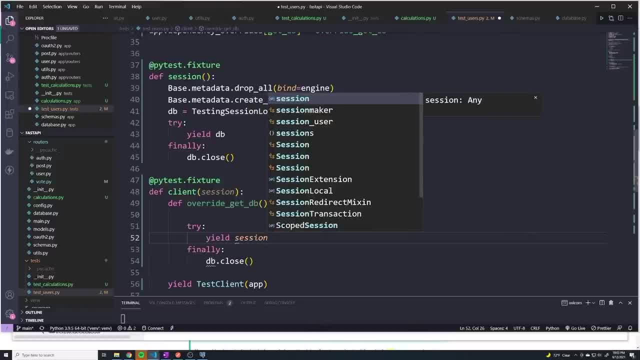 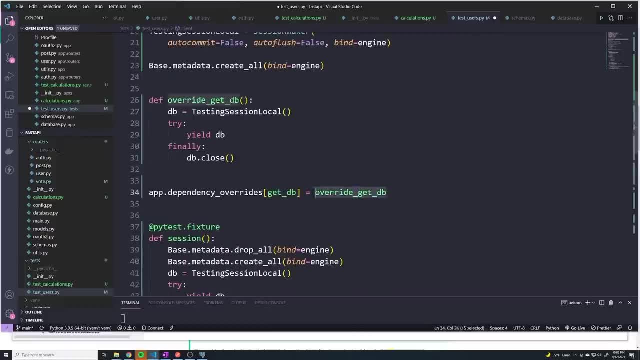 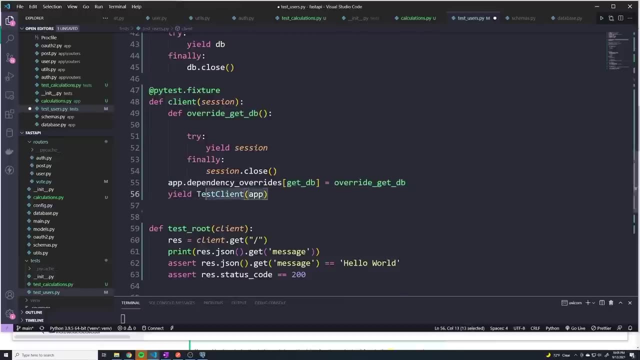 is the DB, So we'll say session And then sessionclose. and I'm going to copy this line right here: Do the override right here, And then we return a brand new test client. Okay, And the benefit of this is that. 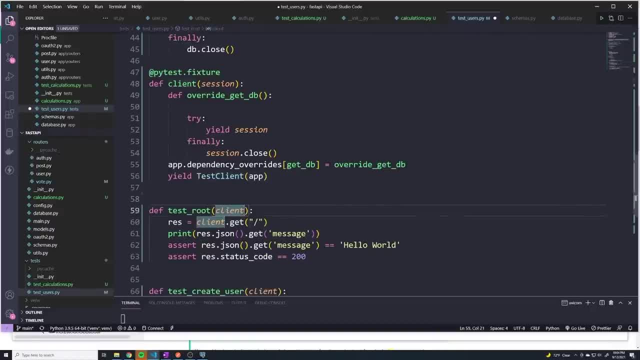 Not only do we get access to the client, If we wanted to, we can also get access to the database as well. So I could say session And then I can go in here and I can make queries like session dot. query, you know, models dot. 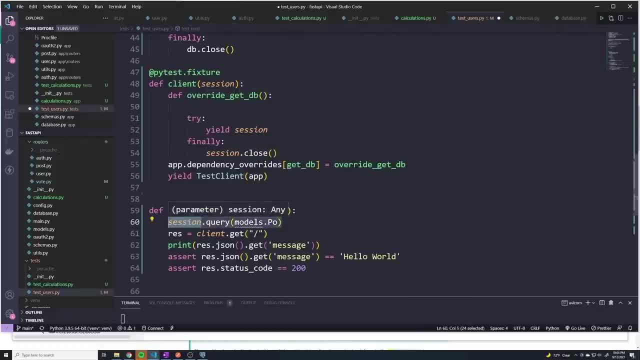 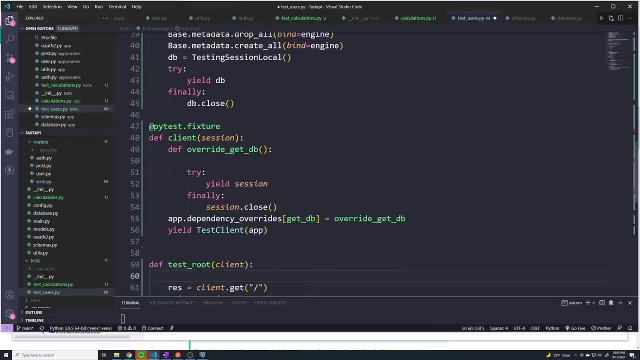 post: blah right. So now I have access to the database object as well And so I can make queries and I have access to the client. But if I call just the client, remember the session database is a input argument into the client fixture. 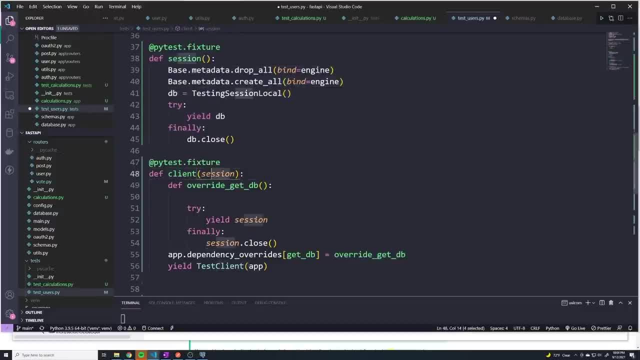 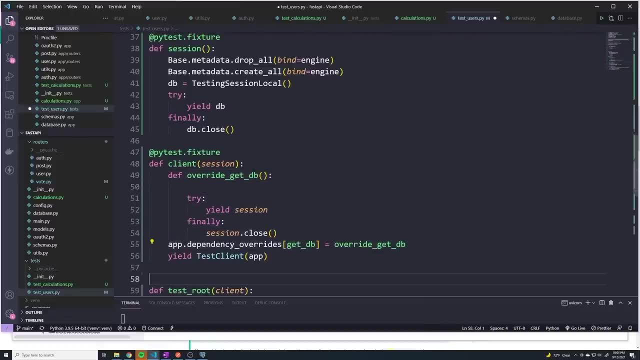 So session will always run first And then client will run, because we're calling it right here, And then we just move the override, get DB function into here as well as the override right here, And then, as usual, we return the test client. 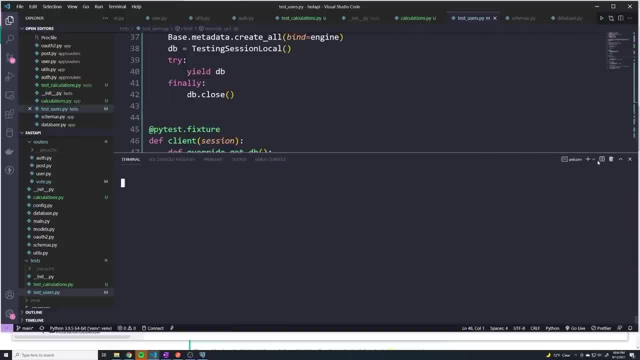 So let's make sure we didn't break anything. Let's test out our code And something's happening with my terminal, So let me open a new one. So let's try this again. I'm just going to do pi test, test slash and then test underscore users. 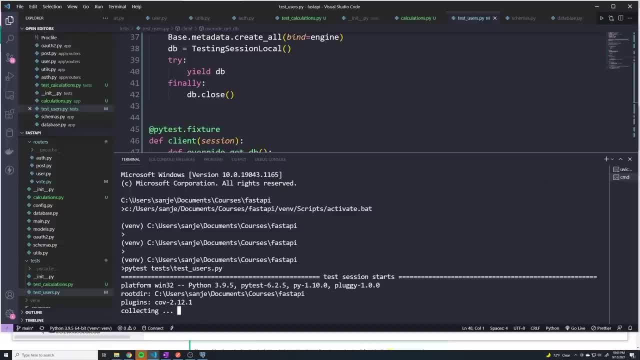 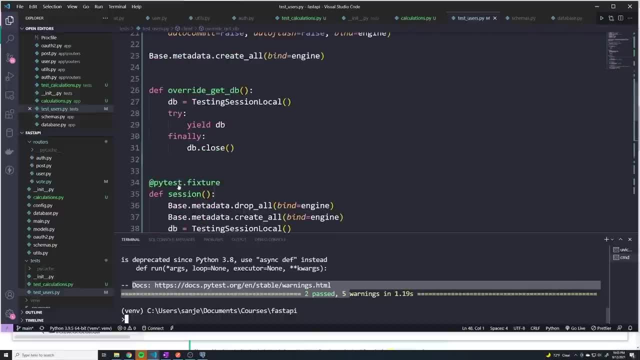 Nope, test calculations, users Alright and two passed, So perfect. Looks like we didn't break anything And we've got a much nicer way of setting up our code. We can actually remove this override that's not within a fixture. we no longer need that. 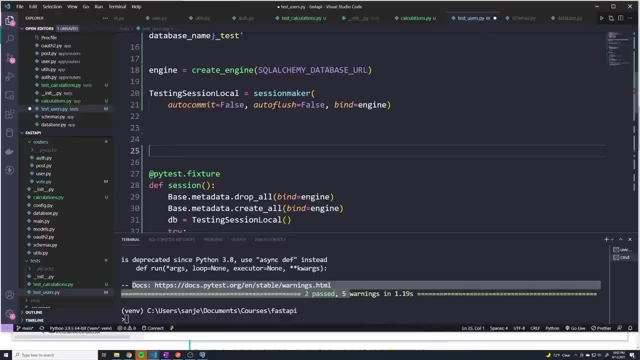 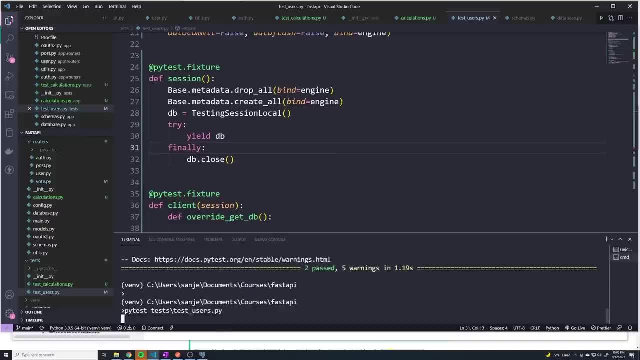 And we no longer need the create all right here outside of any of the fixtures, because we're doing it all within the fixtures now And once again, I just want to make sure I didn't break anything. So let's test that out And we can see to have passed. 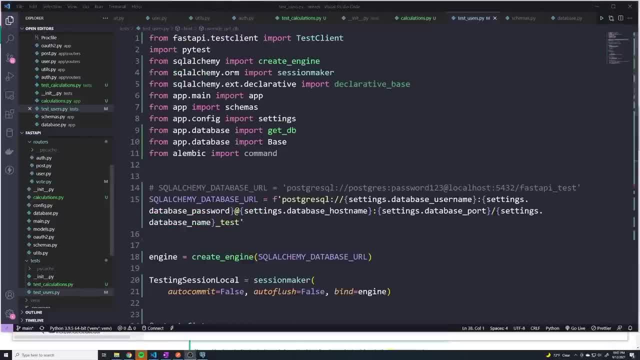 Perfect, Alright. so right now our test users file is a little bit cluttered with all of this data database information And I would like to move all of our database specific code to another file. So under our test folder I'm going to create a new file. 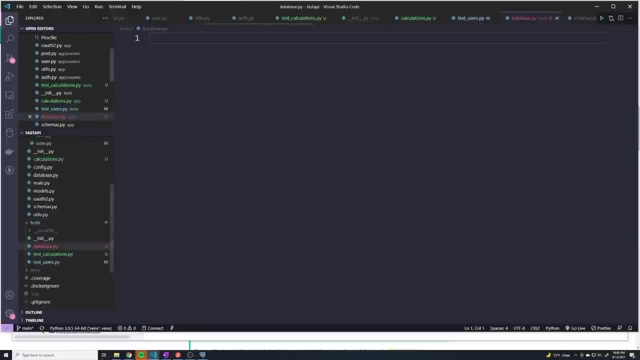 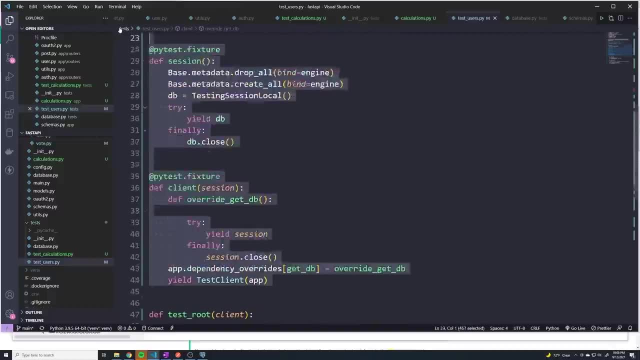 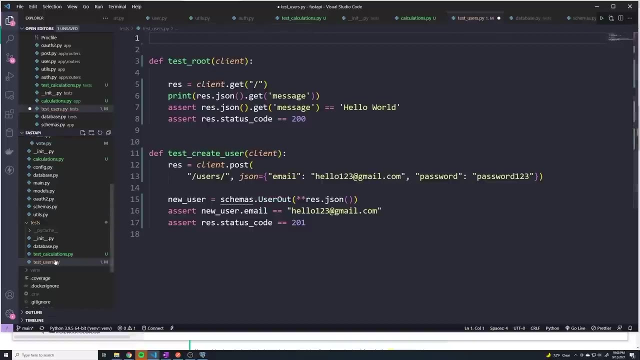 And we can just call this database dot p y, And I'm going to essentially move all of my database code to that file, And that includes the fixtures as well. So these two fixtures, all of this, actually everything. we don't need any of this in our 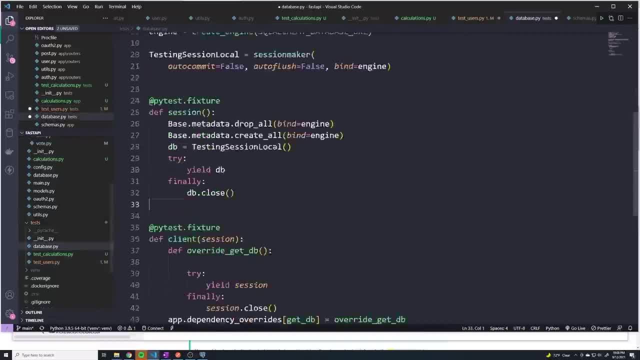 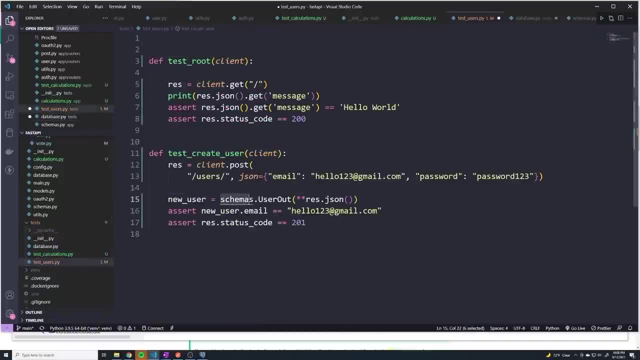 test users file And we can just paste it into here. Now, this is going to break things, because obviously it has no idea what scheme Okay. well, actually, before we do that, we do need to have schemas in here. So let me find where schemas is and we'll just cut that out. 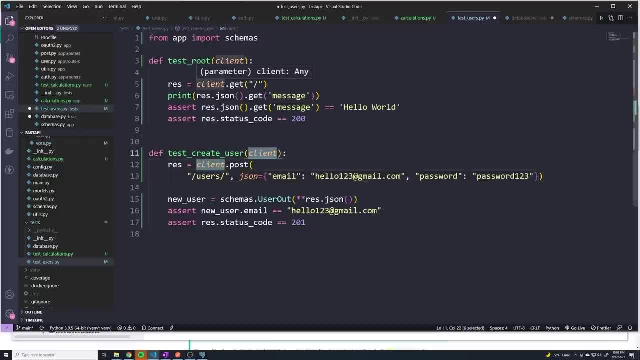 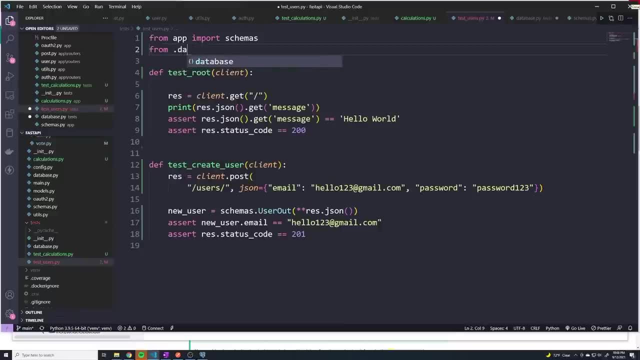 But the other issue is is that we no longer have access to the client fixture, So we have to import that. I'll do from current directory database: import What is a client? I think it's client. Yep, So now we have client. 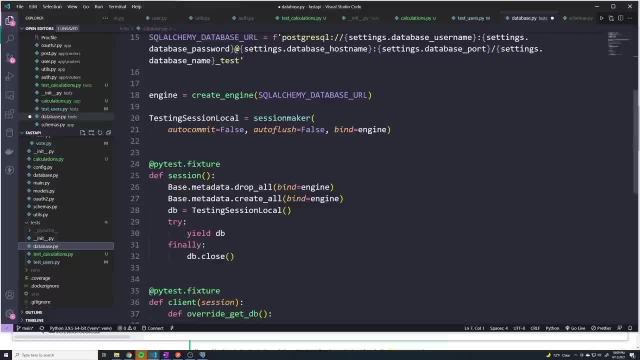 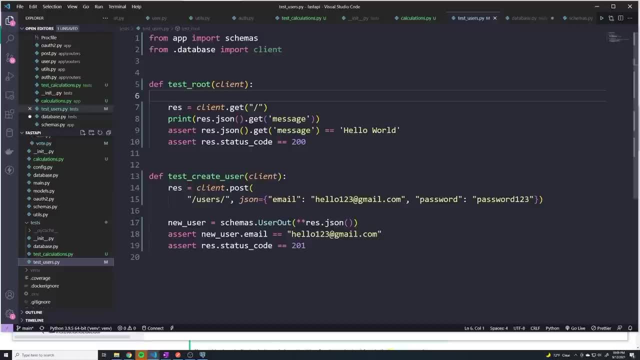 And remember we don't need to import. Actually, we may need to import session. Let's just double check to see if this causes any issues. So let me save everything And let's test this out. Let's see if this works. 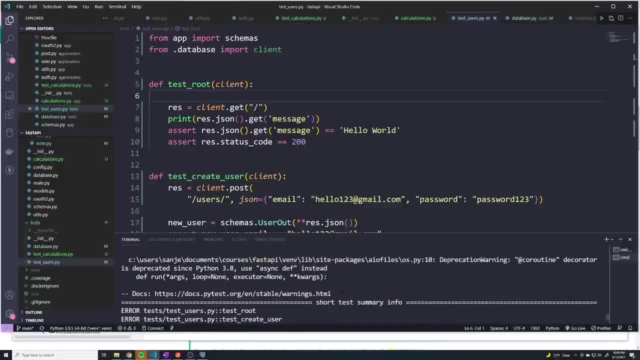 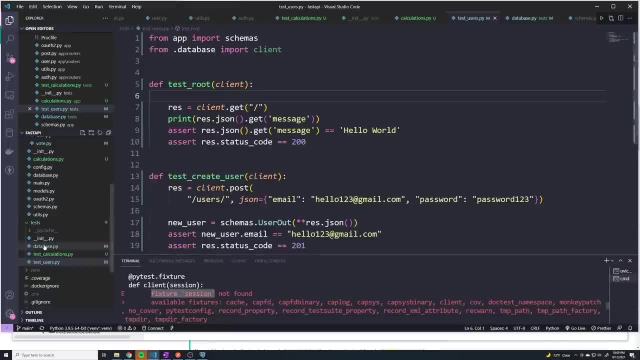 Looks like we got two errors, Yep, And if you take a look at the errors, it says The session fixture is not found. So we actually have to import the session fixture from this file, even though we don't actually call session in here, because client is dependent on session, because client is. 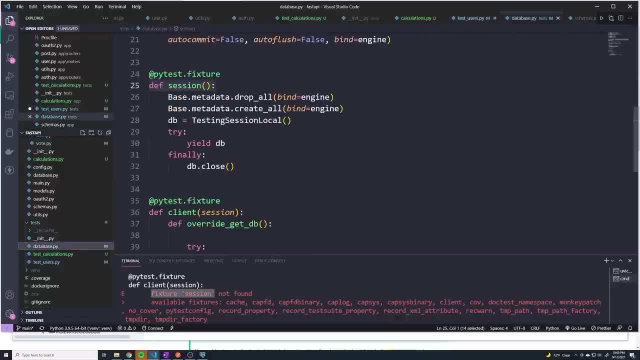 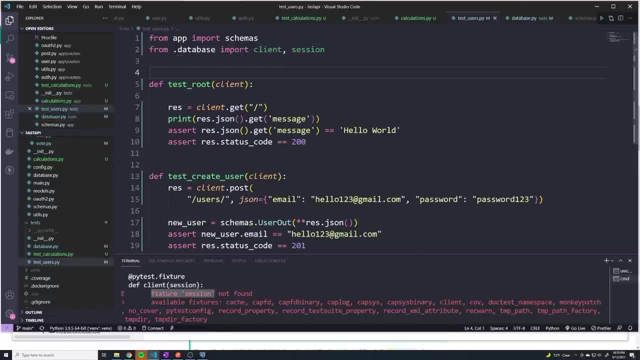 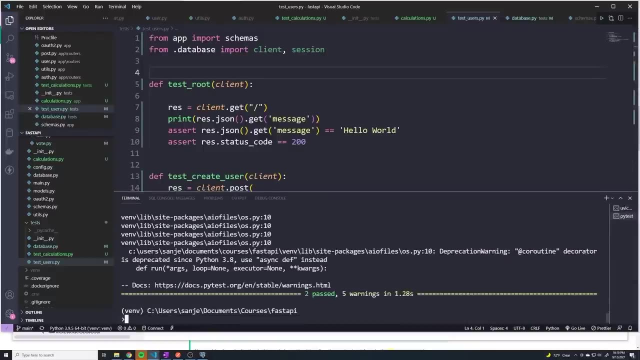 ultimately calling session. we need to make sure that session is also imported, So we have to do session here as well, And so now I think this should fix our issue. Okay, So now, if we run this, yep, both tests have successfully passed. 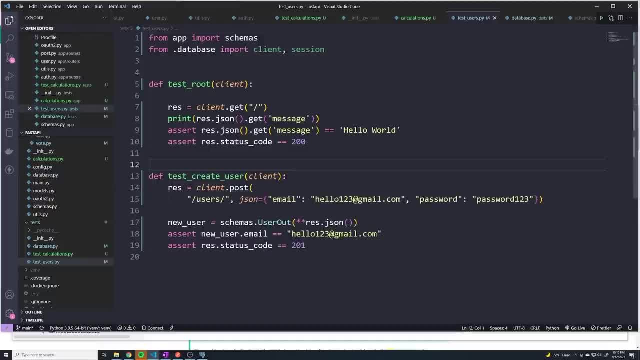 And if you actually take a look at our test file, you can see our test file is a lot cleaner. It's really just got our two tests and a couple of imports And before we move on any further, there's one thing I want to point out and I ran into. 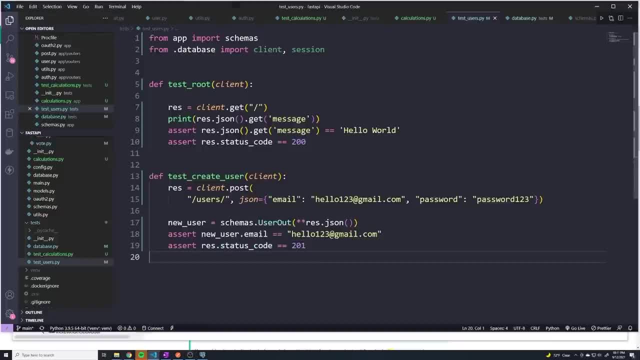 this issue when I was, you know, run doing a dry run through my code. If you actually take a look at your routers- and we'll go to, since we're taking a look at test- create user. this is going to be this slash users. 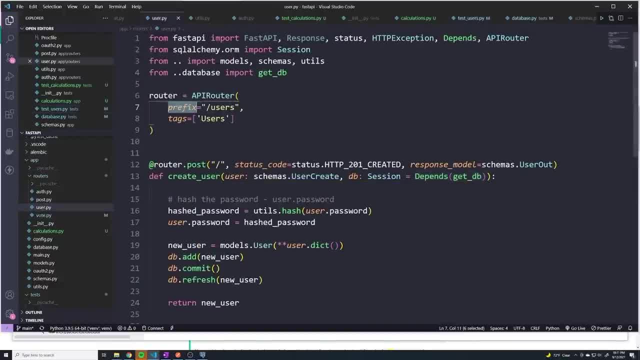 So we go to users and then create user. Alright, you can see that the prefix is slash users. So the route you want to go to is slash users, And then you can see that we have to append whatever's here. So here it's, appending: slash. 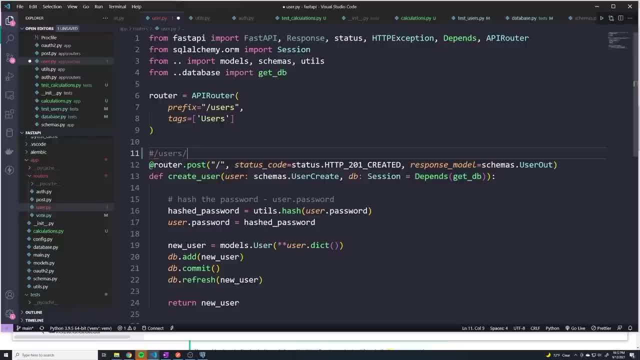 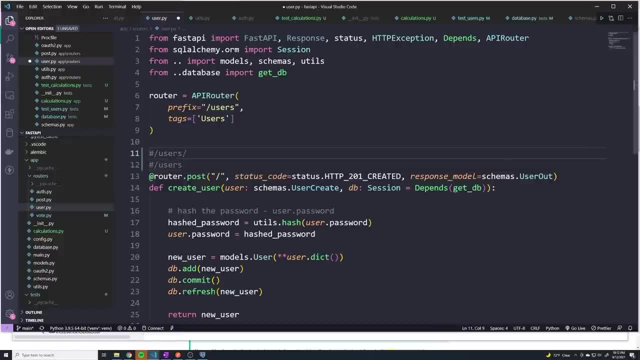 Now the way that pi test works is that, or actually the way that anything works is that if you actually send a request to slash users, it's a little bit different than slash users slash- And I'm actually going to show you what happens when we do that. 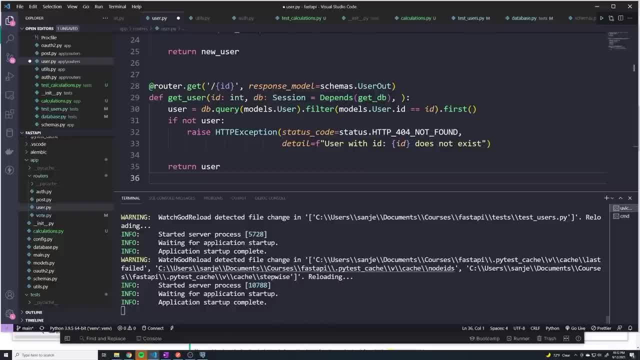 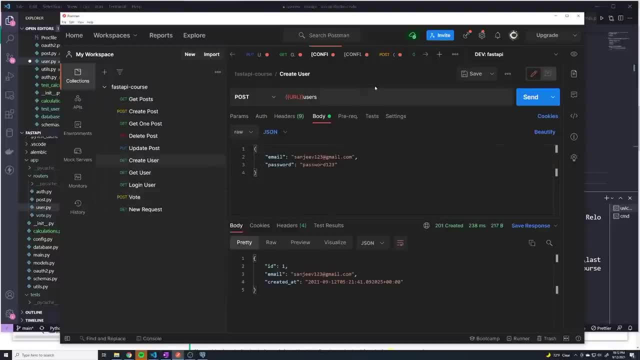 So I'm going to first of all open up a UV coin set. So I've set it up, I start, I started out my API And if we go to create user here, I'm going to users and not user slash, right, I'm not? 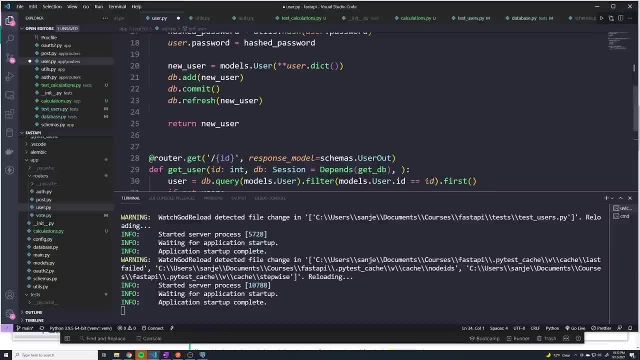 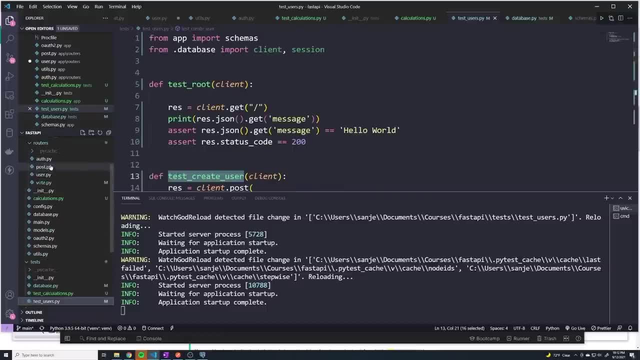 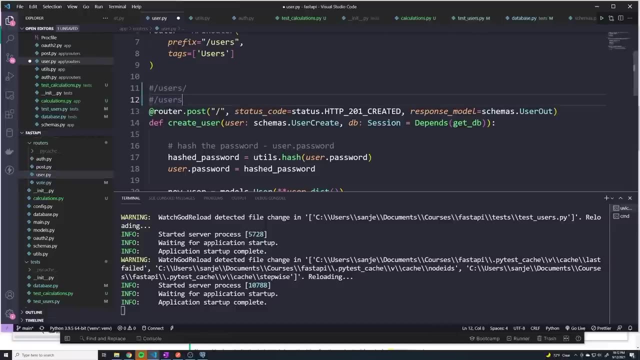 doing slash. I'm doing slash user. I'm just doing users, which is where did it go here? Where did I put my the things I just typed? let's Yeah here. So what we're doing is we're sending a request to this one, not the one above it, because 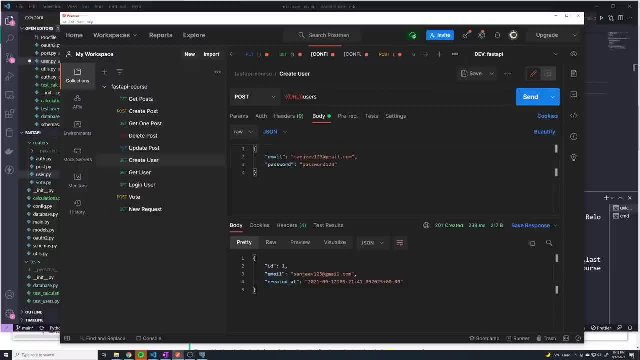 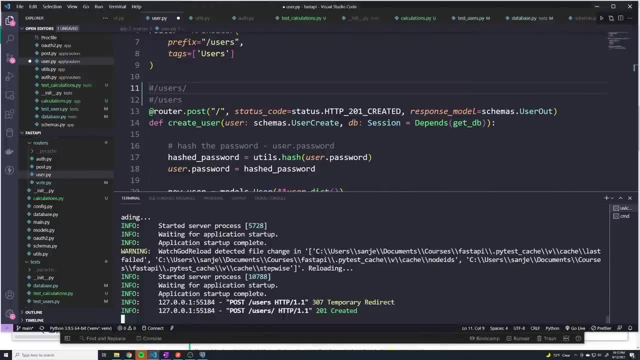 the other one above it, It has a slash at the end. we don't have that trailing slash. So if I create a test user without that trailing slash, hit send. Take a look at what happens in the logs. it says that when we get a request to slash users, 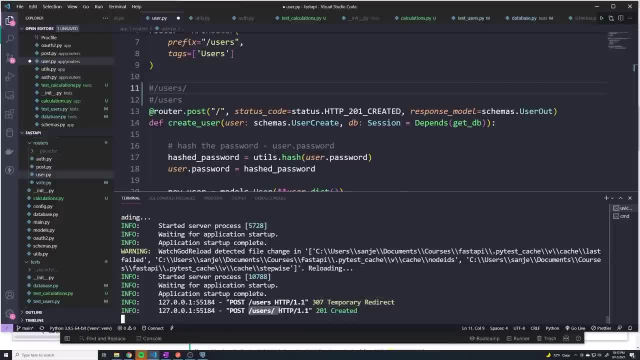 we're going to send a 307 redirect to slash user slash because technically the routes on slash, user slash and fast API is intelligent enough to actually send the redirect to here. However, this creates an issue with our testing, Because if I just do slash, 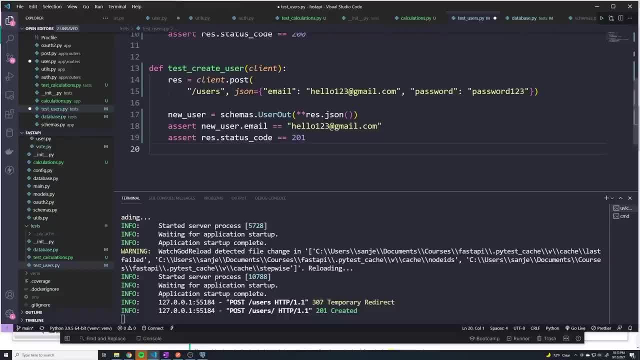 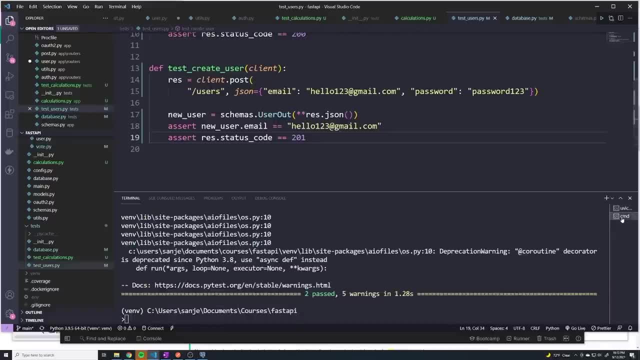 What's going to happen is, when I do this res dot status code check, it's going to check for 307 and not the final 207, the final 201.. And I could show that to you guys. So let me go down here. 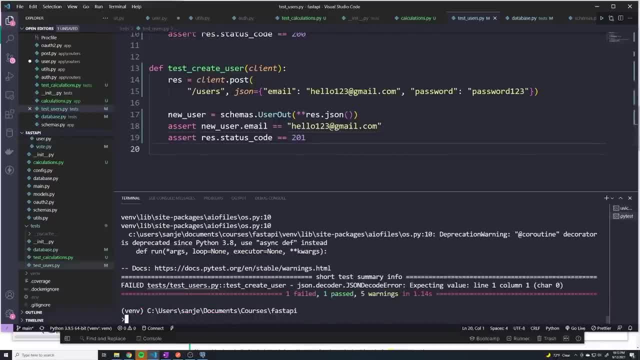 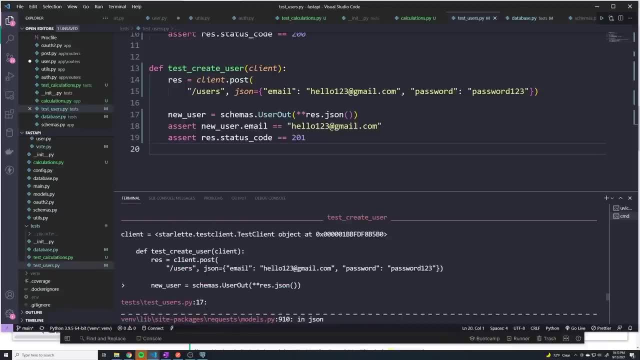 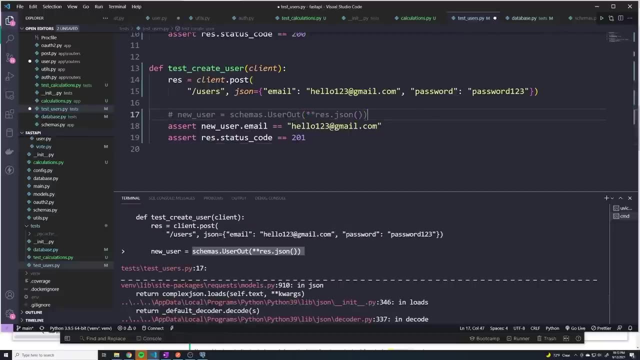 We'll run our test real quick And you'll see that it fails. and it fails because, well, there's a couple of issues It fails. It's. it says it fails because our validation for a schema failed. I'm going to skip that and comment that out. 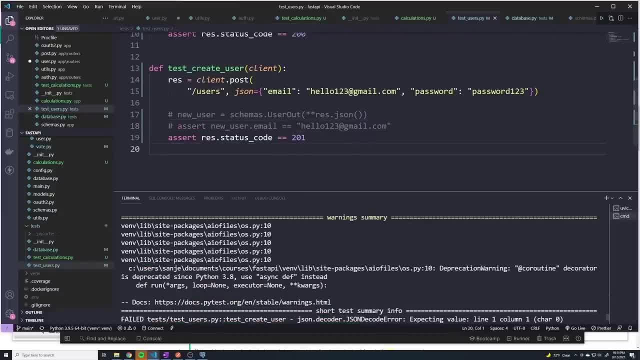 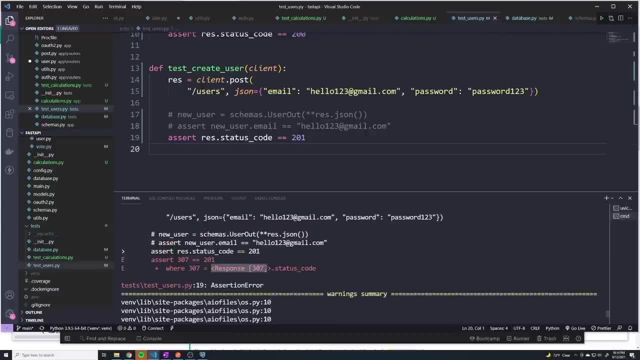 And I'll comment this line up. I just want to take a look at the status code Because obviously, if there's a redirect, there's no information in there And you can see that this fails because the response code is 307.. 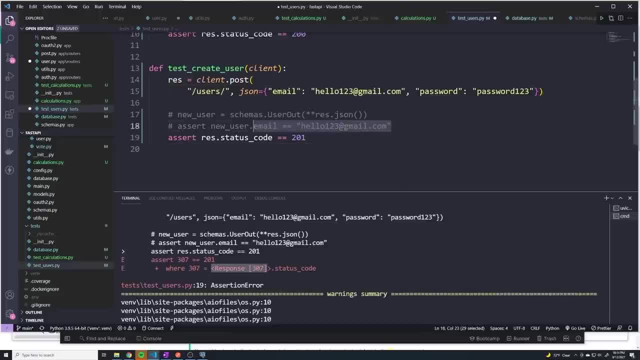 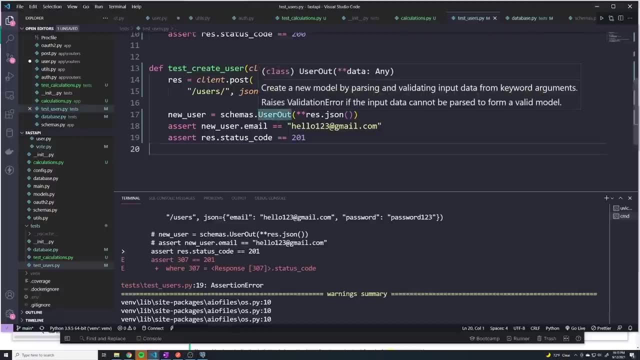 So that's why you want to make sure you add that trailing slasher. then you'll run into some issues. So we've got our create user test pretty much done. You can feel free to customize it however you want. If you want to add a few extra cert statements, feel free to do that. 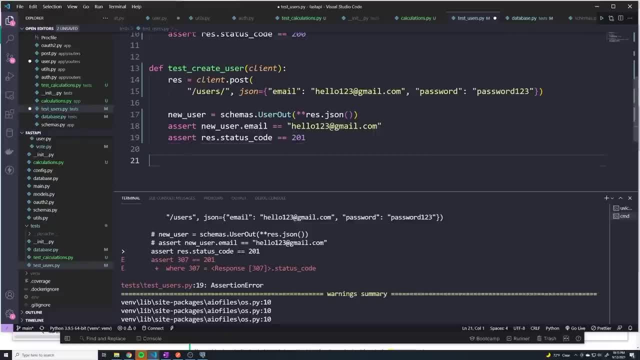 But we're going to move on to login. So let's actually handle setting up the login. So I'm going to do def test: underscore login, underscore user: Alright, and this test is going to be dependent on the client fixture, because we need to be. 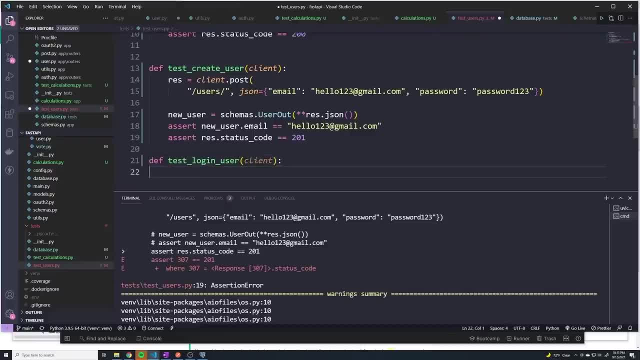 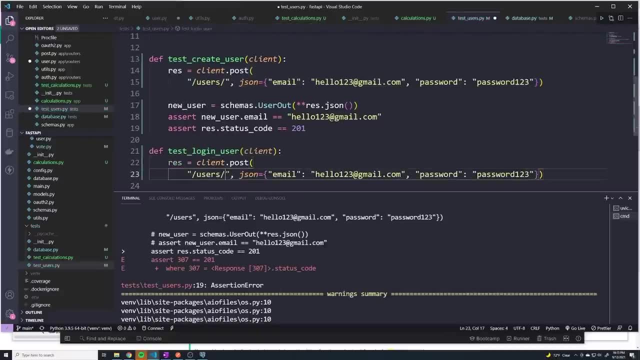 able to send a request. So I'm going to pass in client And I'm actually going to copy this line right here. We'll change it, of course, but alright, and so we're going to. this is going to go to slash. 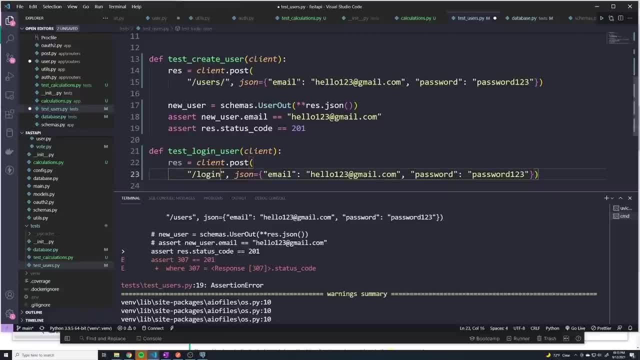 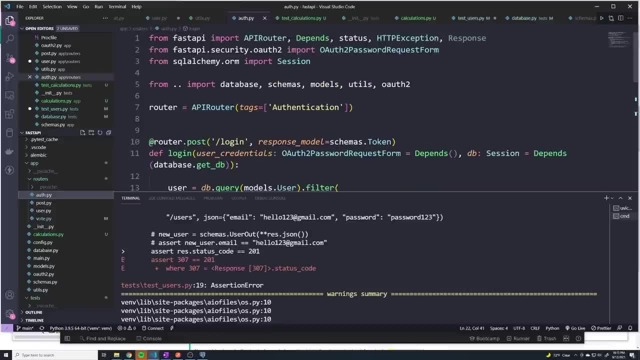 login And there's no trailing slash on this one. Just because if you actually look at our specific route for login- I think it's under authpy- You can see there's no prefix here, It's just slash login. So we don't need the trailing slash on this one. you just have to figure out how you set. 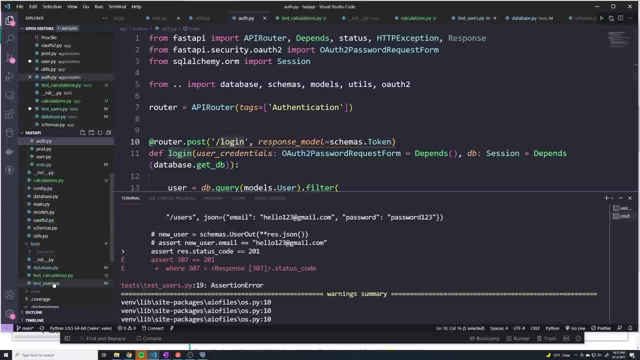 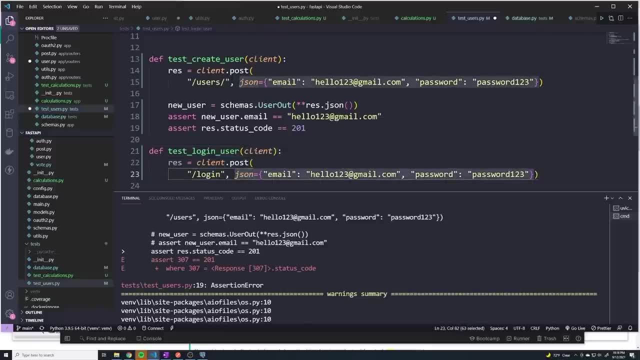 yours up and make sure it matches accordingly. We do slash login, But in this case we don't want to send this data in the body. Instead, remember, if you go to postman and you go to login user, we don't send it in. 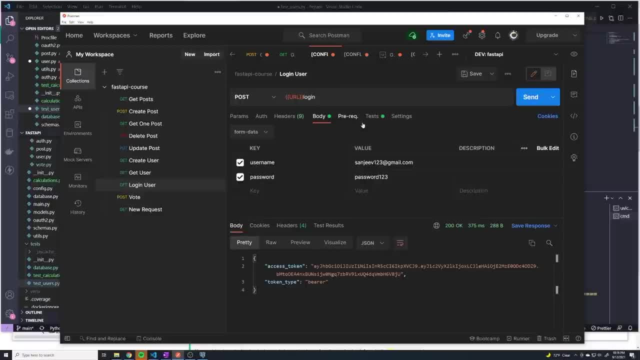 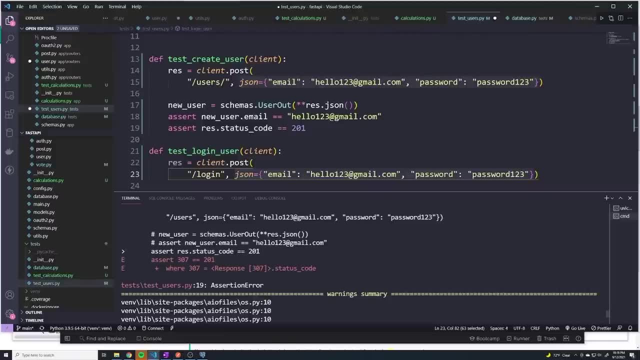 the well. we do send it in the body, But instead of using The normal, normal JSON format, we have to send it as form data, remember. And so to change this to be form data, you just change JSON to be data. 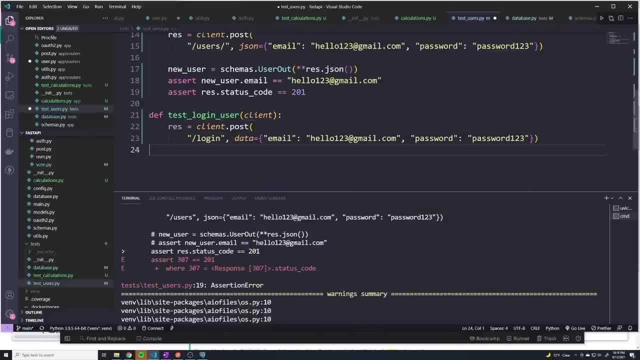 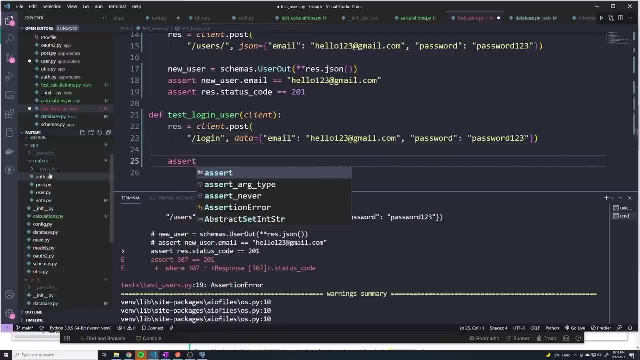 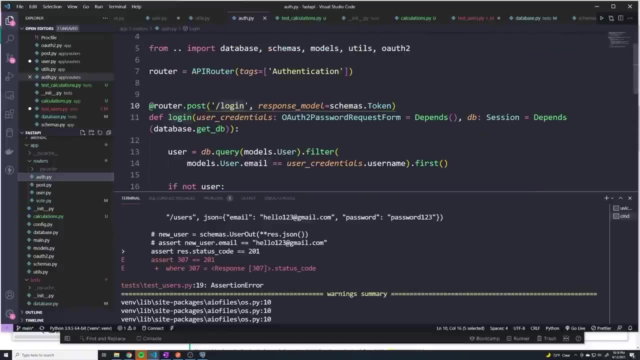 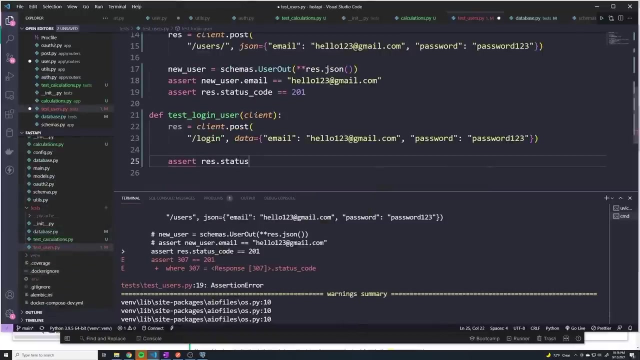 And we've got the same credentials, So this should work. Let's just quickly just do a assert. And what is a login return? A login returns a. It should just be a 200.. So we'll do a 200.. Assert- res- dot status code. 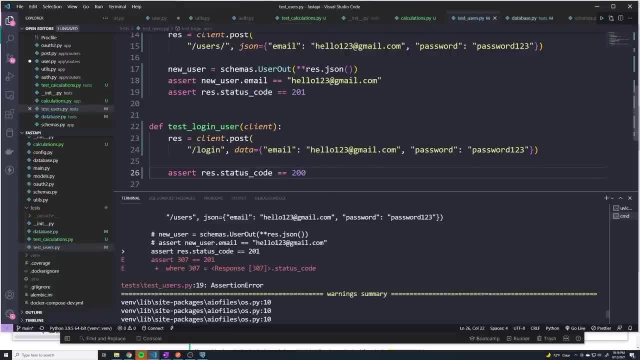 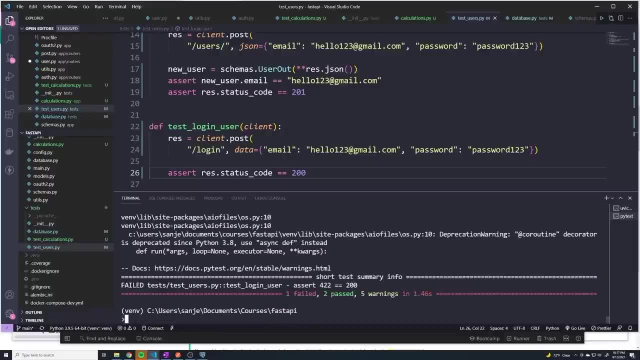 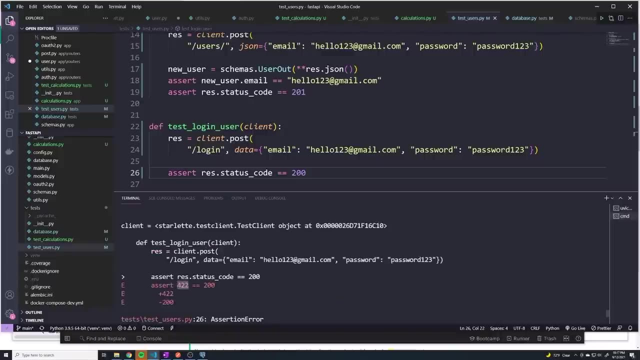 Equals equals 200.. All right, and let's test this out now. And it looks like we got an error. So what happened here? Let's take a look. It looks like we got a 422 as our status code. Why would we get a 422?? 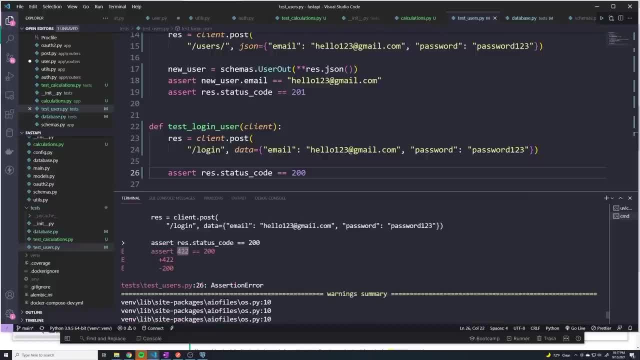 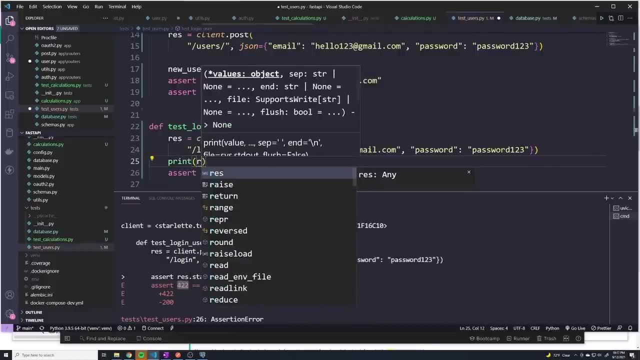 And if we take a look at our logs, we don't really get much information here. So what I'm going to do is we're just going to print res dot JSON so we can see what's going on. Why did we get a 422?? 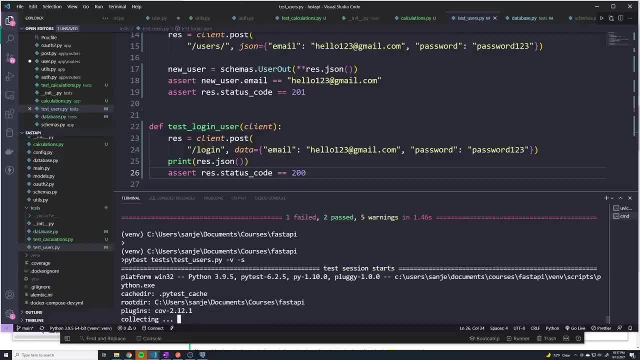 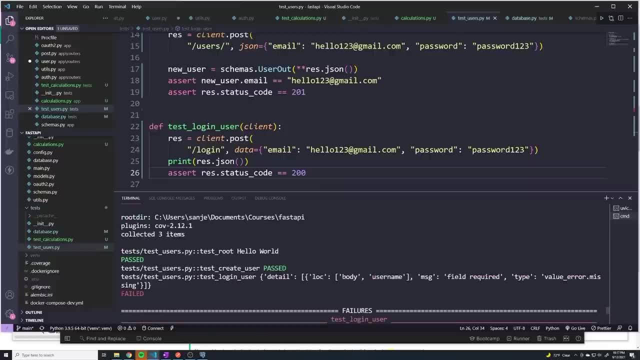 Is there any other details it's going to provide us? So I'll do a dash s So it prints it out And we can see in the print statement it says: Oh, look at this, there's some sort of validation issue. 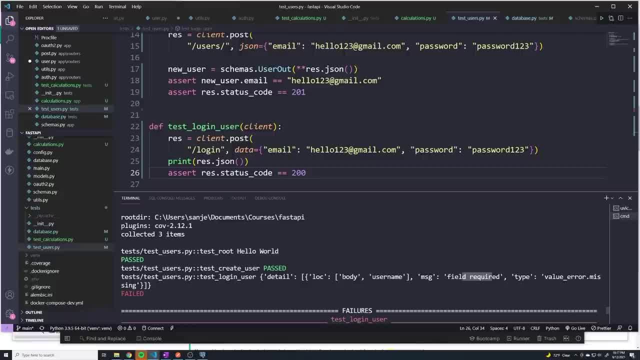 We have a bug. It logs. We washed our hands of this. We've got this real good here and we can't read this. We don't really see it, but it's going back And it links back to our notice here. 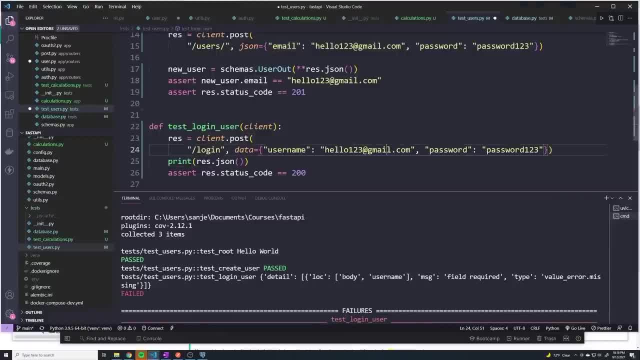 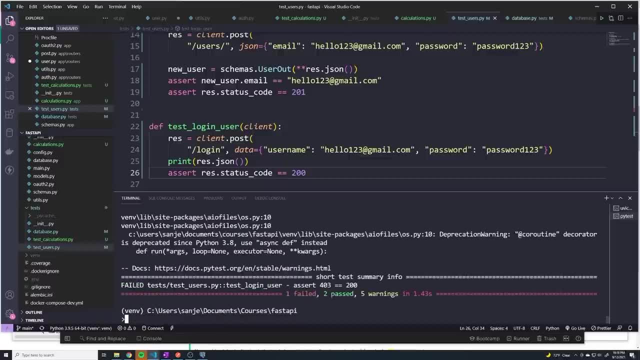 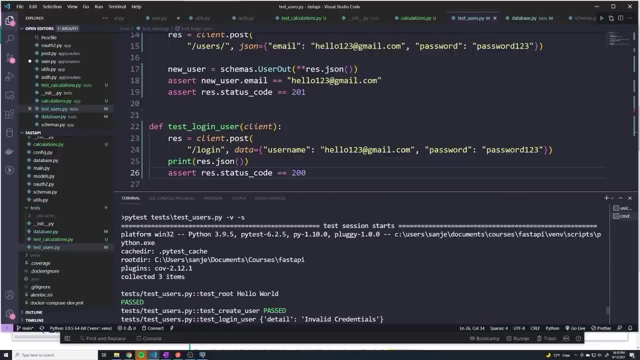 We just pulled this data candy from our data, So our log status has a smear which is shown to be a complete error. All right now we're just checking that out on our log. Does that change anything? Sure interesting. So what's happening? Why did we get a 403?? Let's see. Detail says invalid. 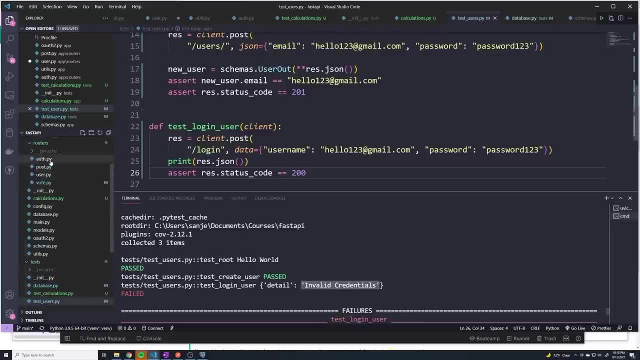 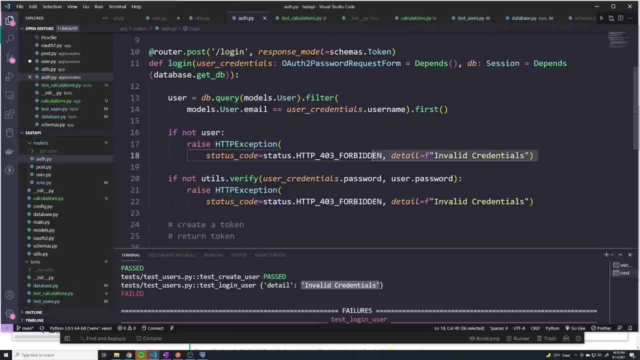 credentials Interesting. So if I go back to my login route, right, you could see that we get a a 403 if the user doesn't exist, which means we couldn't find a user with that specific email, or if the password that was provided doesn't match what's in the database. 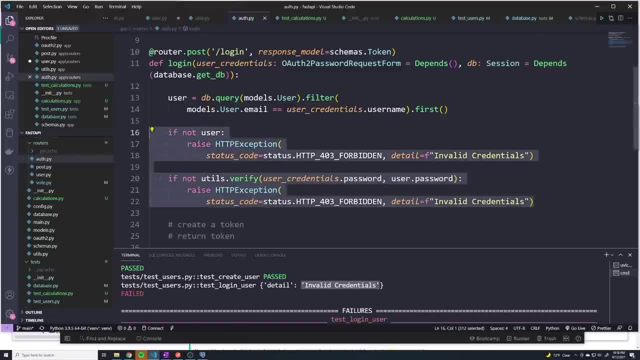 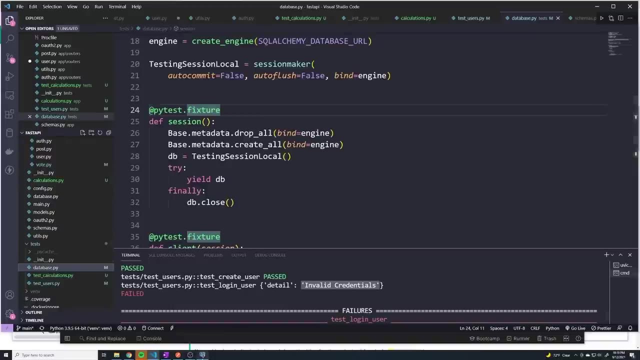 So this is one of the issues. it's either the user doesn't exist, or the email doesn't exist or the passwords incorrect. So let's go into PG admin And if you left your your database config so that you don't drop it at the end, instead you drop it before a test case starts. 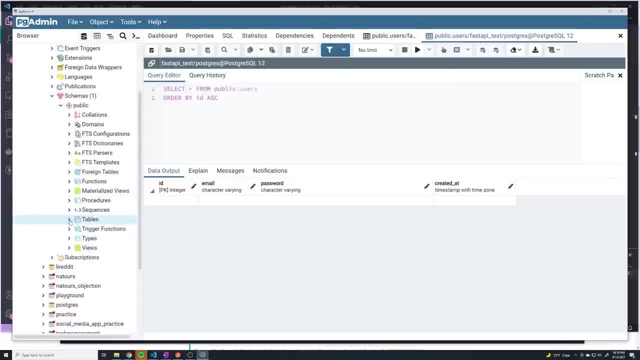 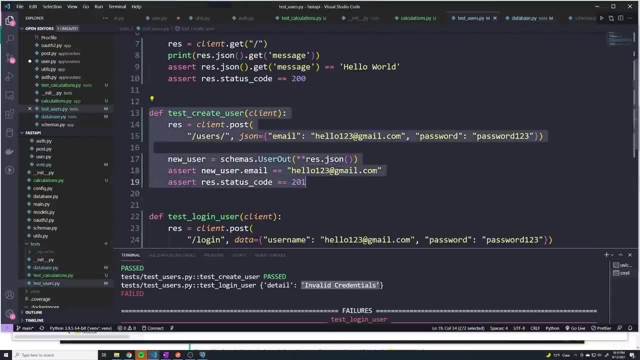 you should be able to see all of your test data. So I'm going to refresh this. And if I go to users view, edit data, all rows, right. well, there's no users. Well, that's interesting, Right, Because if I go to my code during our test, create user we should have created. 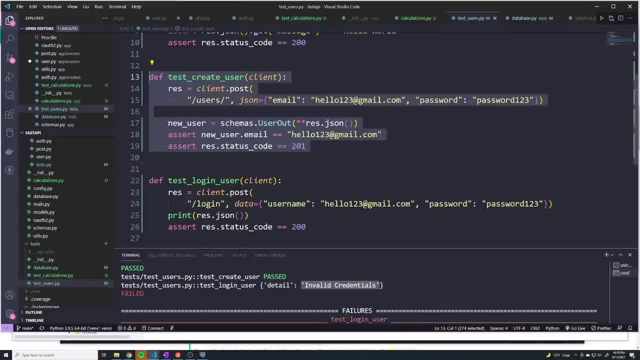 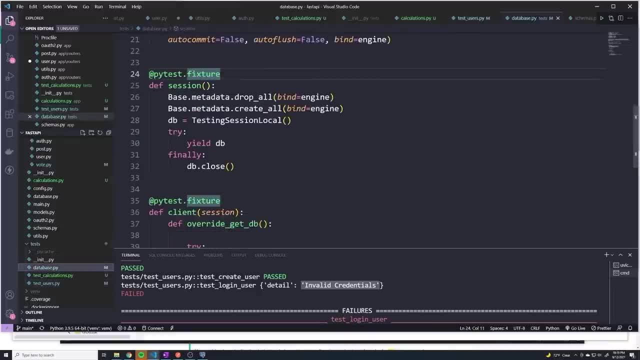 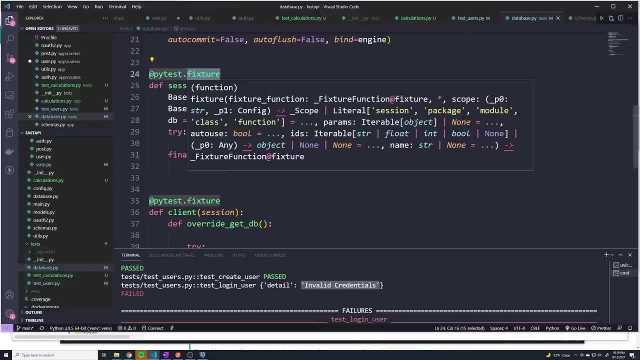 a brand new user, So why can't we log in as this user? Well, that's easy to explain. So if I actually go to my, my database, dot p y, we have these fixtures And the fixtures have a specific scope, which means when do they run? And right now they're using the. 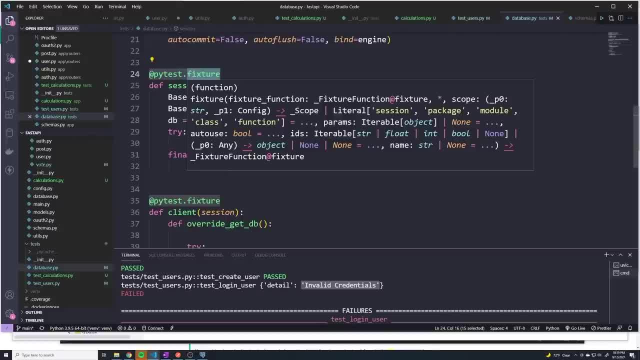 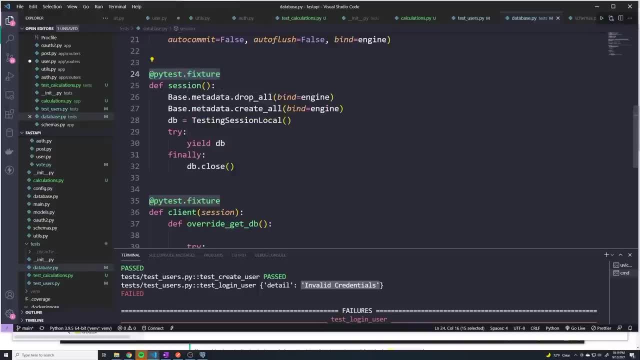 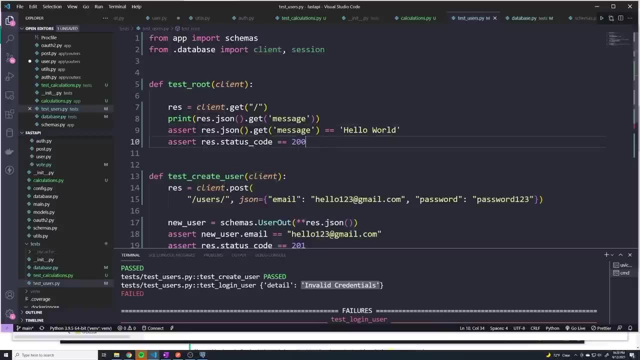 default function scope. What that means is they're going to run for every, they're going to run before every single function that's dependent on them. So that means when we run test users right, we can see that test route client Right. 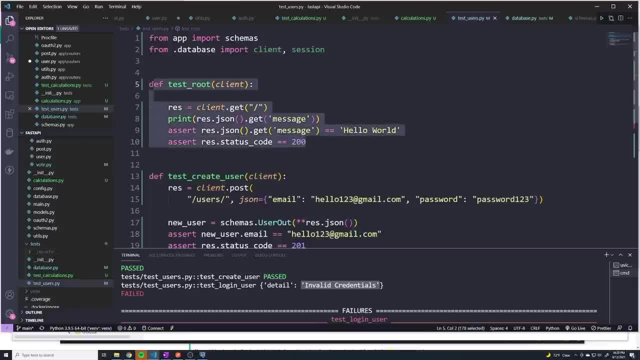 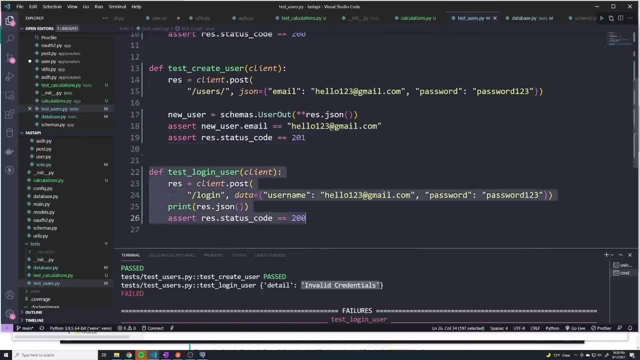 Since we're passing client into test route, we're going to run our fixtures before we run this function, Then, before the next test, we're going to run our fixture again, And then, before this test, we're going to run our fixture again as well. So why does that? 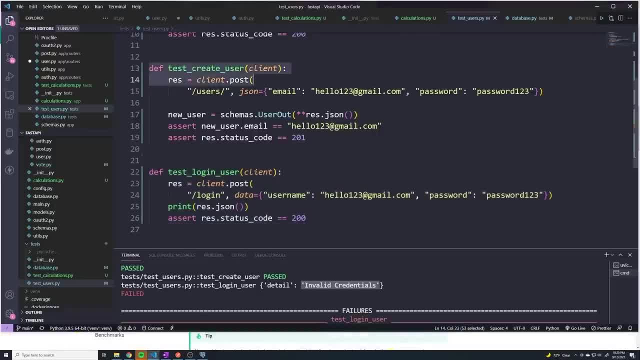 actually cause the user get deleted? Pretty simple, Because we run this test right, The test create user, the users in the database, and then we start to run the test login user. And so, since we're dependent on the client fixture, we go to the database, dot p y file. we can see that the client calls. 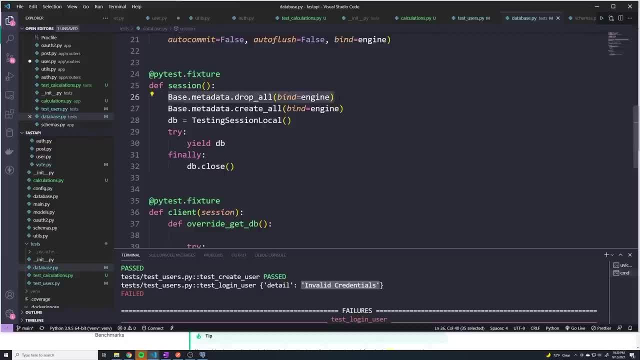 session session. what does session do? Well, it drops the database, or it drops all the tables at least, And then it creates a all of the new tables. So we get a brand new database every single test that we run. 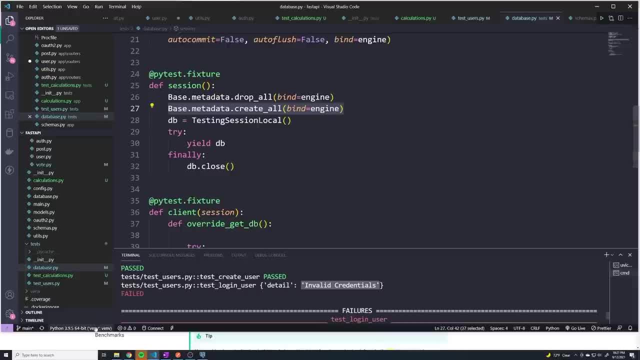 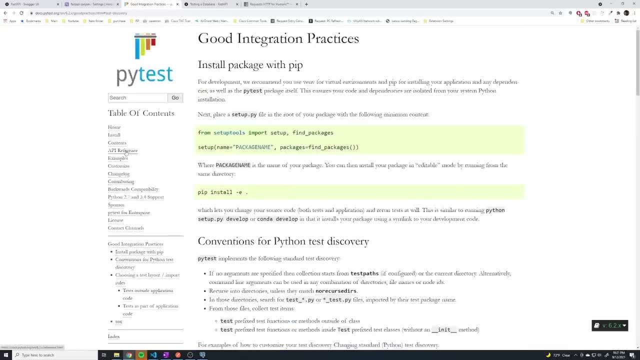 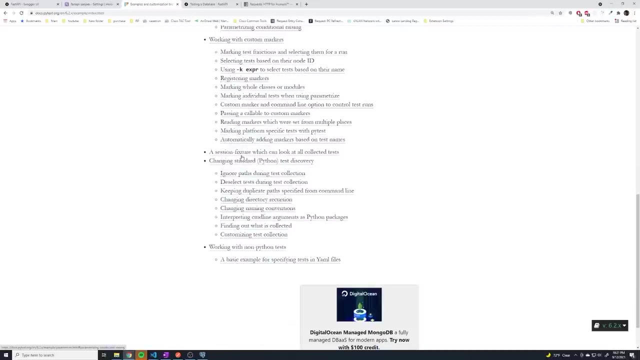 That's why the user isn't there. And if you want to learn more about scopes, I recommend you go here, And then, I think, I go to API reference, I think, And then fixtures, Not No, let's go to examples And go to fixtures. 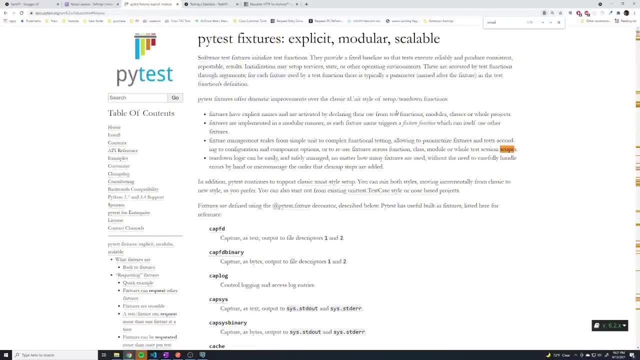 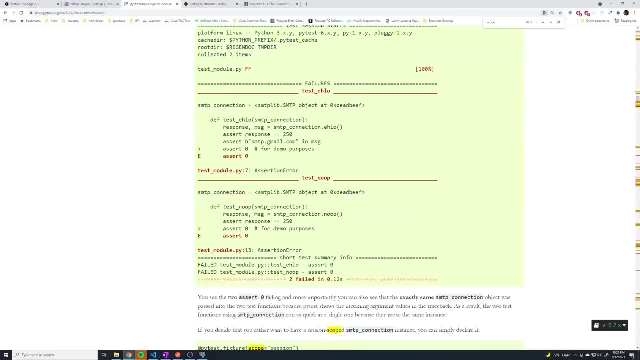 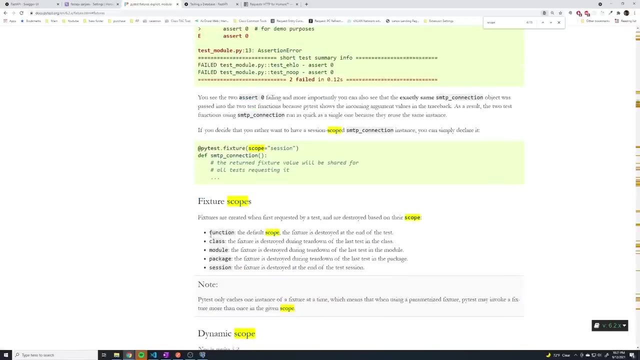 right here And then here I can search for scope. Here we can see the different scopes. So the default right now is that our scope is functions, which means that the fixture is destroyed at the end of each test and it's run for. 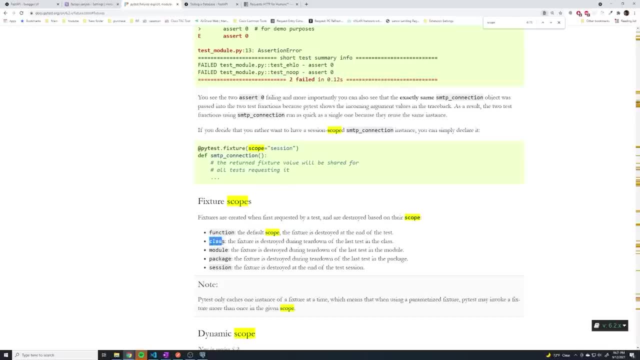 every single function. we then have a fixture that sets to a scope of class, which means that it'll run once per class, And it'll run once per class, and it'll run once per class, and it'll run once per class. 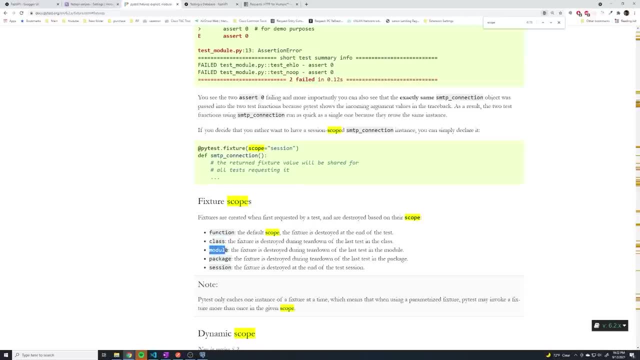 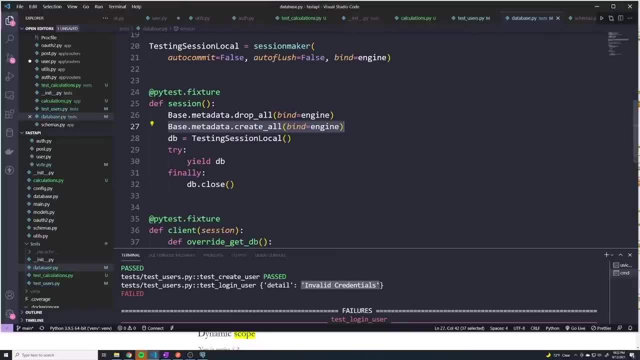 run all the tests in the class. then we have a fixture module. So when a fixture is set to a module, that means for all of the tests in a specific module, right, like in this case, all of the tests here. we're going to run the fixture just once at the beginning. 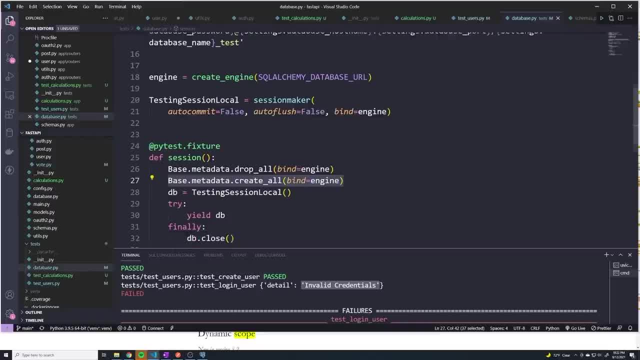 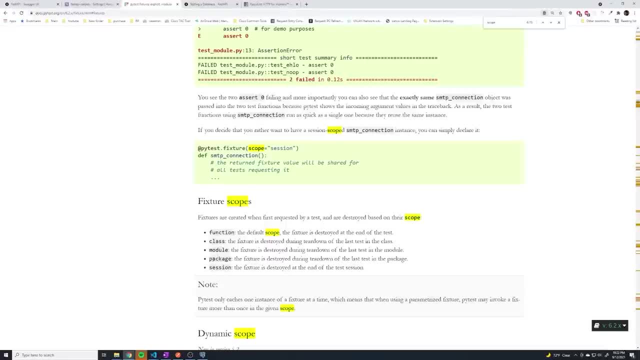 And then we're not going to run it again for that module. So all of the tests will have access to just that. first instance run essentially, And then we also have it for package, where it's going to run once per package, And then 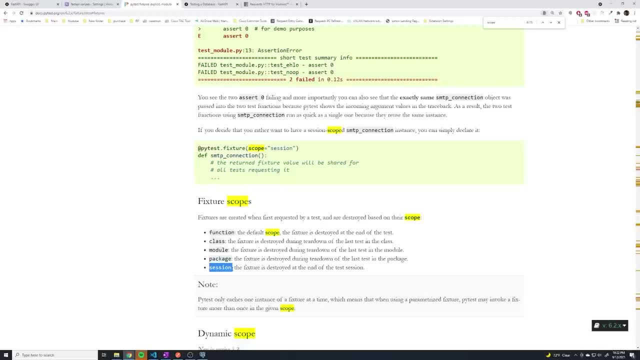 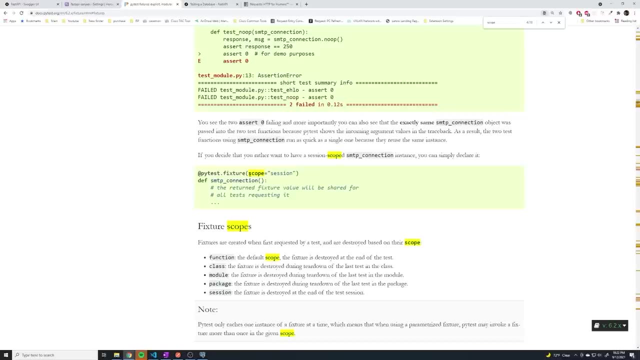 we also have session where it's going to run once At the start of the testing session and it's going to get destroyed And you can see how we can set the scope right here. you just do scope equals and then whichever one you want. 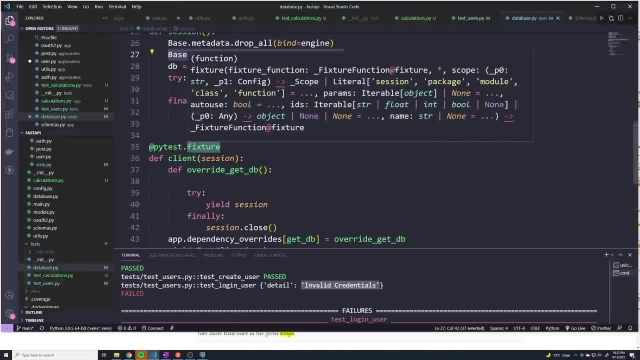 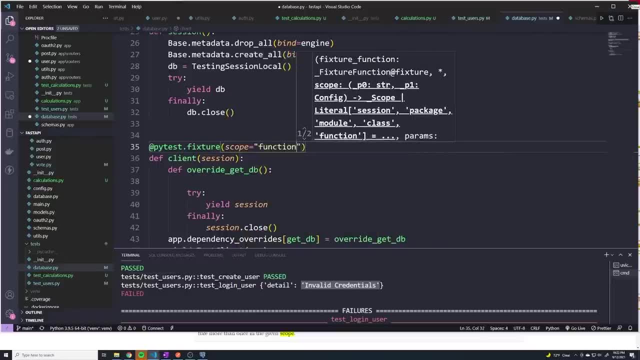 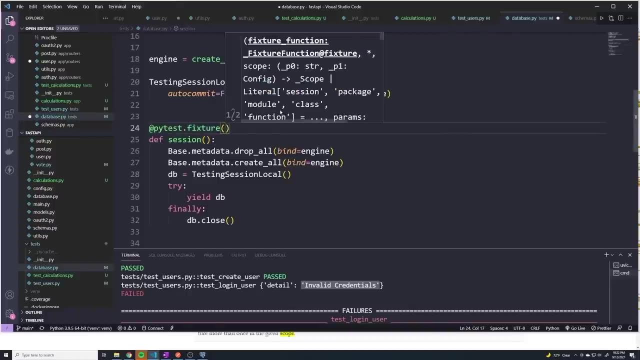 So if we go back to here and we see this, this fixture right, we could say, since the default is function, it's the equivalent of doing: scope equals function, And the same thing goes for the session, the database one as well. So these are going to run and get destroyed every single. 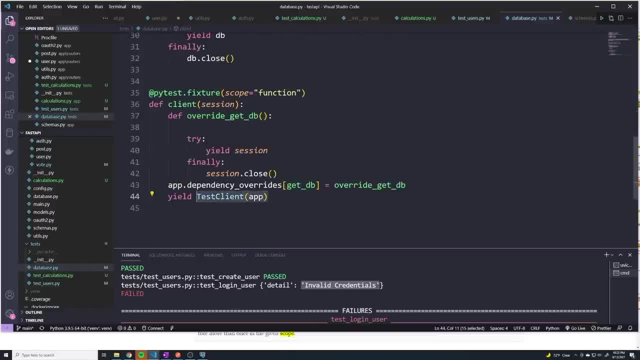 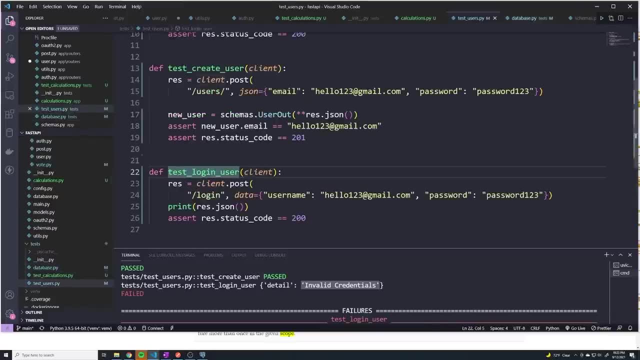 function. So at the end of the function, we're going to delete this test client and then we're going to create a brand new one for the next one, which causes our database to get wiped and destroyed. So if we want our login user to be able to access what was created, 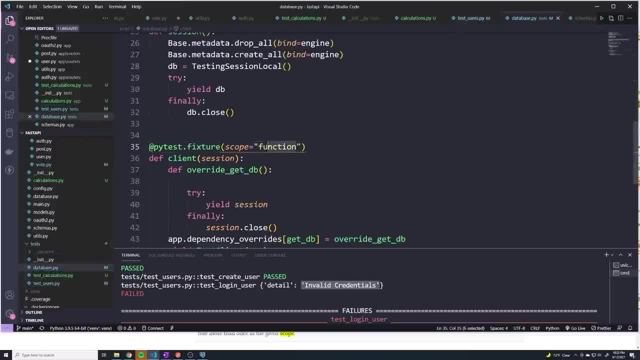 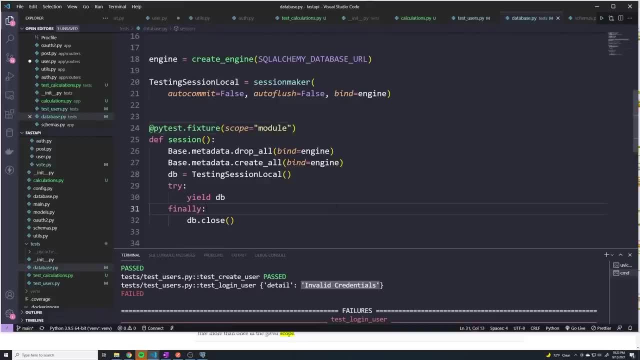 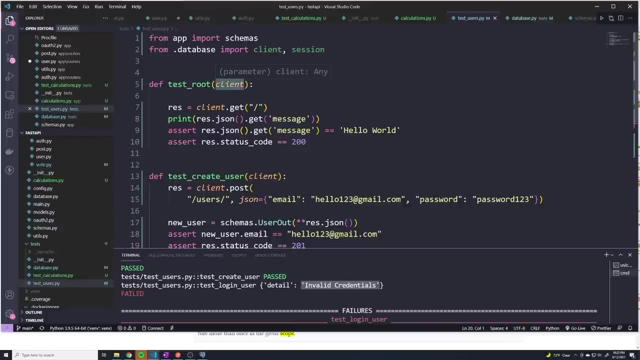 here we could theoretically change the scope to be module instead, And we could change this for both. So now what happens is at the start of this module, when we start running the test here. we're going to run the fixture right, Because the test root is calling it, So we'll run. 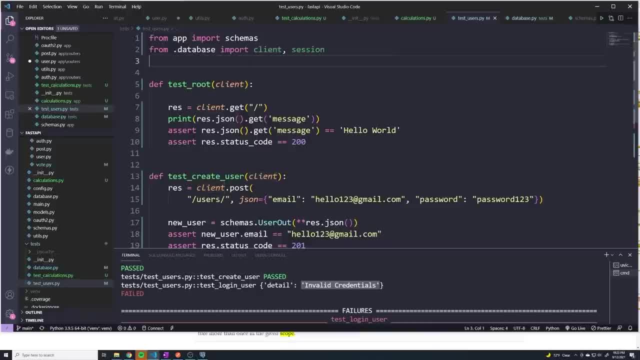 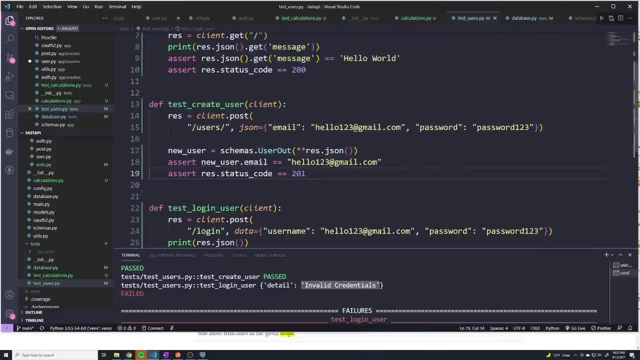 the fixture at the beginning And we're going to just do it once, right? So then we all you know, we'll call this one, which doesn't really do anything. we'll then create the user, But since we don't ever run, 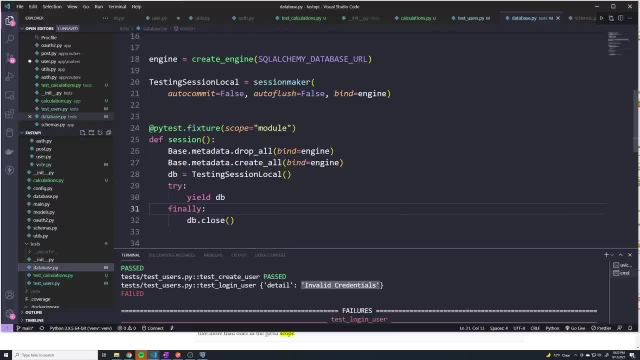 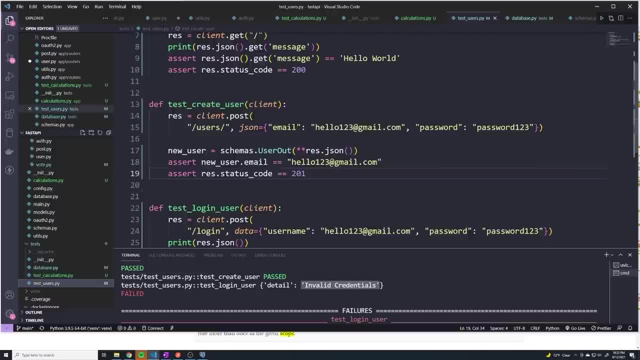 the fixture again. we never end up running this session either, So we don't end up dropping our database database or our tables. So we'll actually keep that same fixture and then we'll run through all of our tests and only at the end will we destroy that fixture. So we have essentially 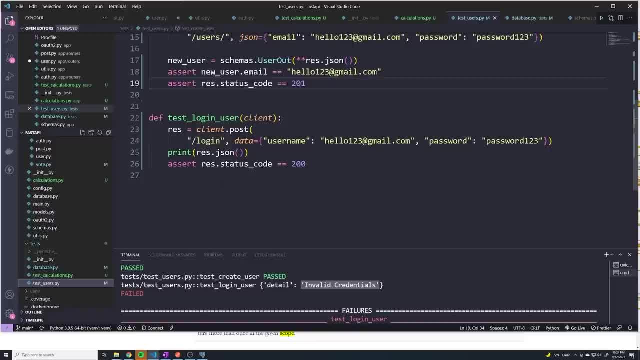 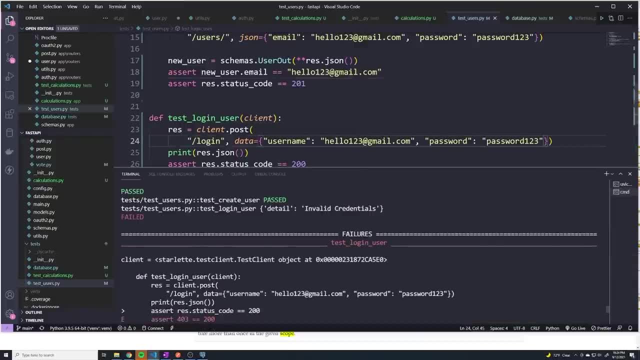 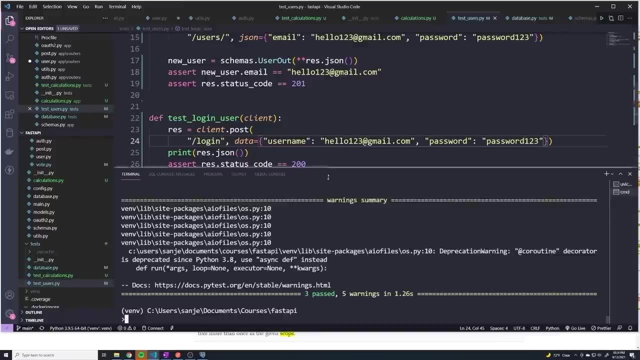 access to our database for the entire module in this case, And so now, if I actually run this, you can see all of our tests passed, because the fixture will last the entirety of the module. I could even use package or session- both of them would have worked, But 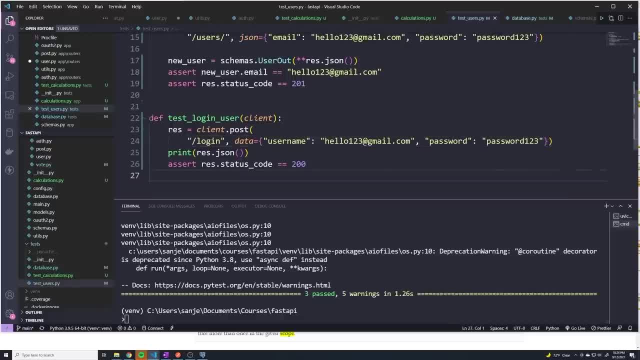 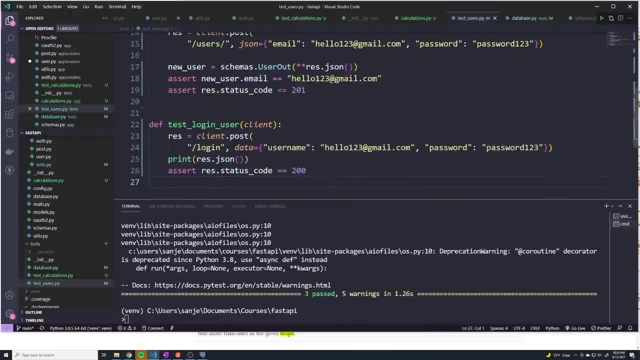 this creates a little bit of an issue because this means that this test is dependent on this test completing. So if this test fails, then obviously this test is going to fail and it actually creates issues because if I move this to the top and I accidentally 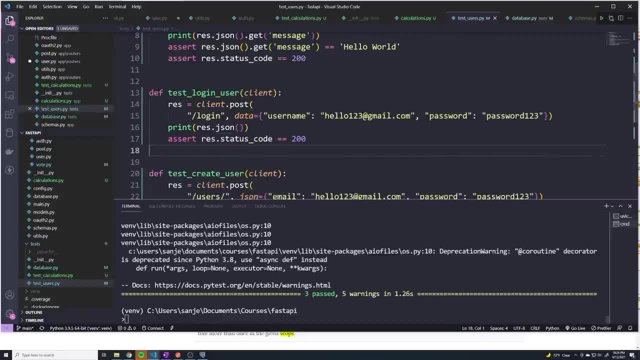 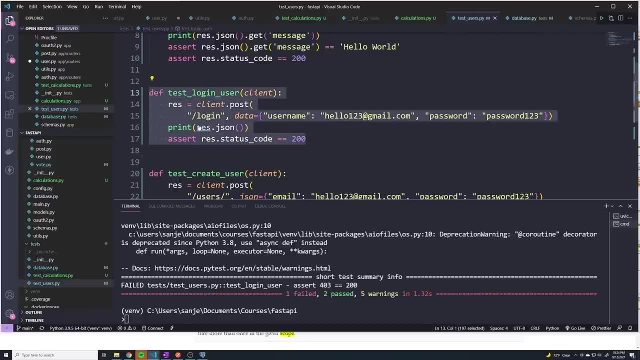 move my login user to before test create user, then this is going to break our tests once again, because we need to create the user before we log in, And so, in general, what we've done is bad practice. You don't want to make tests be. 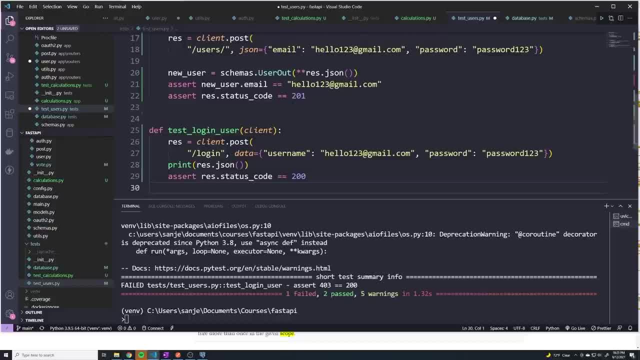 dependent on other tests. Each and every single test needs to operate and run independently. They should not be reliant on other tests. If they are, it is not a valid test and you're doing it wrong. You want to make sure that all tests can run independently of one another. 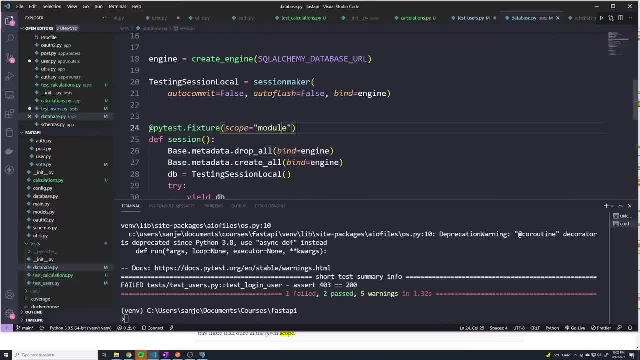 So what we've done so far with this little hack of changing the scope to be module is not a good solution. So in the next video we'll take a look at what we can do to kind of overcome this limitation, this issue, so that we can make our login test case independent of our create user test. 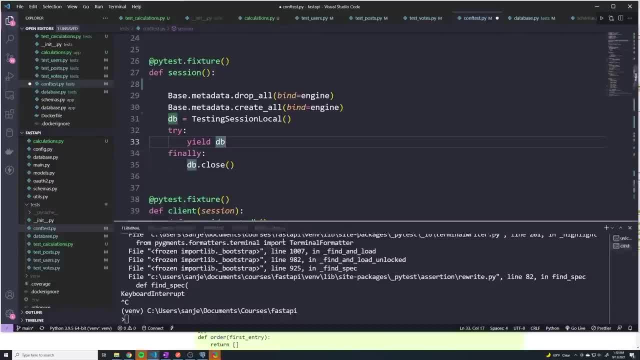 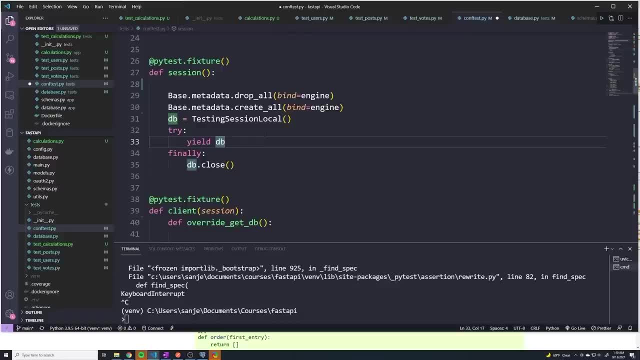 case. Okay, guys, I wanted to make sure that you know we really did understand what scopes are when it comes to fixtures, because I feel like I didn't do that good of a job explaining it. So hopefully this video will help explain it a little bit more. And all I'm going to 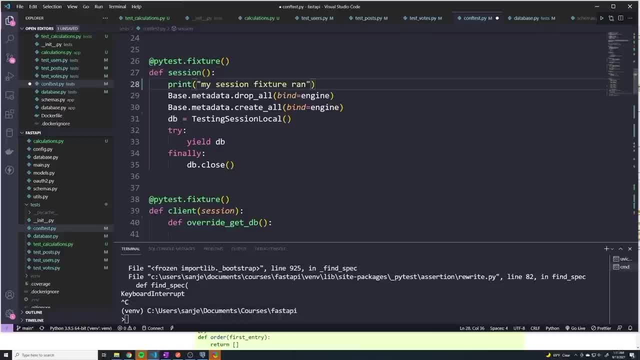 do is under our session fixture. I'm going to just do a little print statement. I'm going to do a little print statement right here that says my session picture ran And this is. you know, I'm recording this video in the future, So I've got all of the other tests. 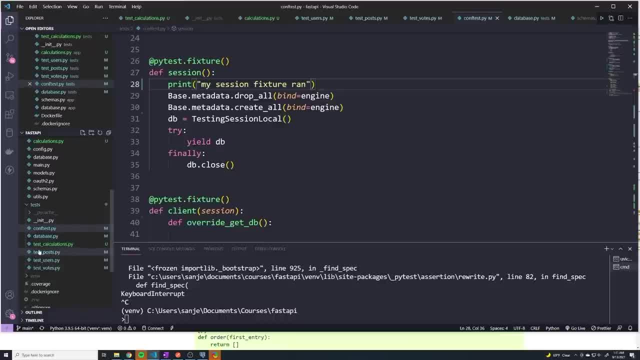 that we're going to cover done already And I've kind of broken it down into test posts, those testing, all of our post path operations. we've got one for users and one for votes. I'm going to show you guys what happens when we use the default scope, which is scoped. 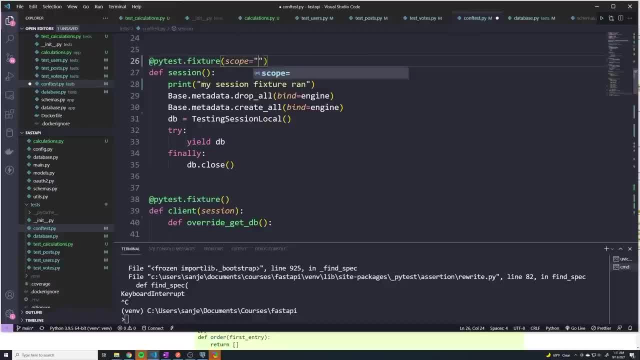 per function. Right, this is the equivalent of doing: scope equals function, which means that we're going to run this fixture For every single time function that requests it, And so if I remove this, because once again it's the default, 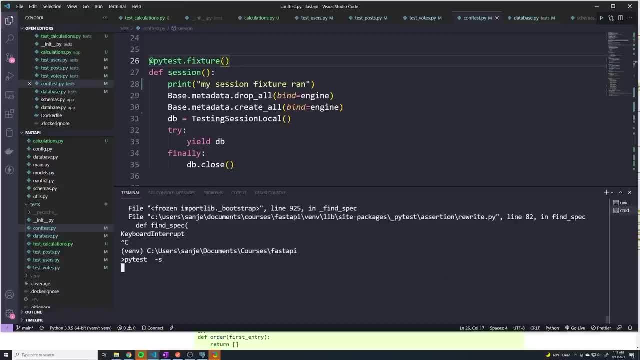 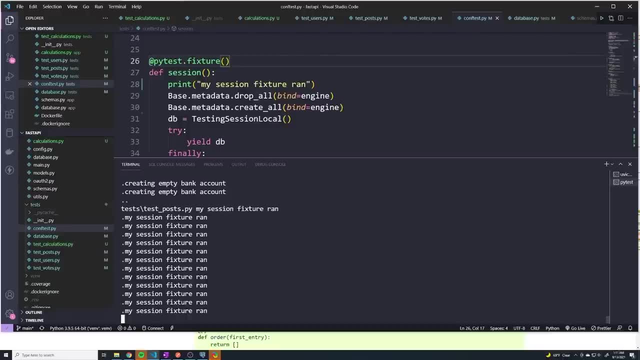 and I run my tests. I want you to take a look at what happens. For every single test that we run, one dot represents the test we can see it prints out, And so it's running through all the tests and tests underscore posts and then it's going to. 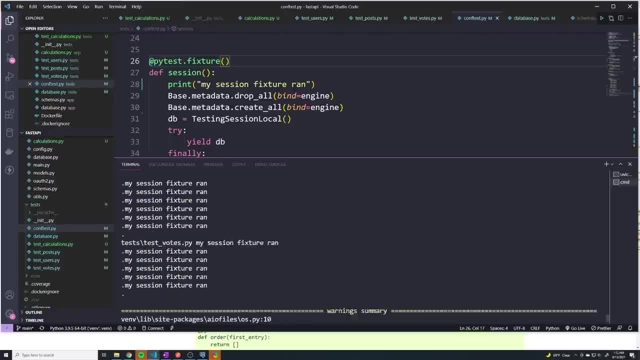 run all the tests under in test, underscore users and then votes. So you can see that, because this is set to function, we're going to run this entire session fixture, this function, every single test that we have, or at least every single test that's requesting this specific fixture. That's why we 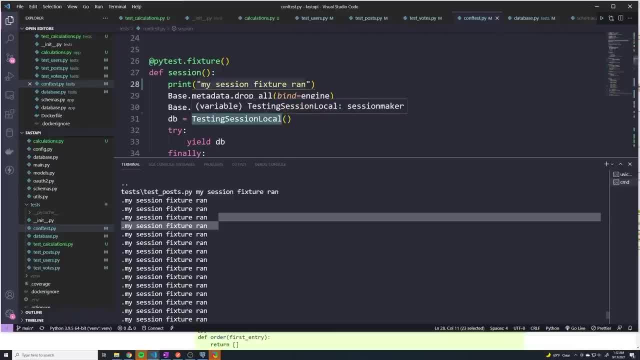 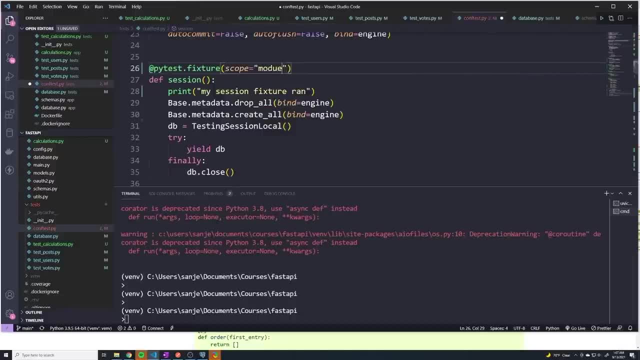 see it run every single time. Now, if we change the scope to module, the behavior is going to be a little bit different. Now, if I change the scope to module, what's going to happen is that for every module that has a test that's requesting this specific 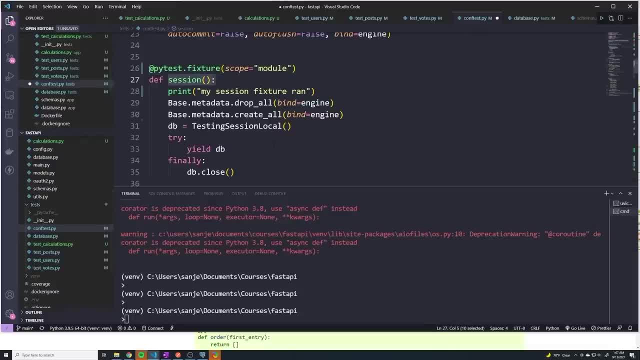 session fixture. we're only going to run this fixture one time per module, And so now, if I save this and I'm going to no longer do dash v, I'm just going to do just dash s, So we can see this get printed out without too much extra data, because we're going to see a lot of tests fail. 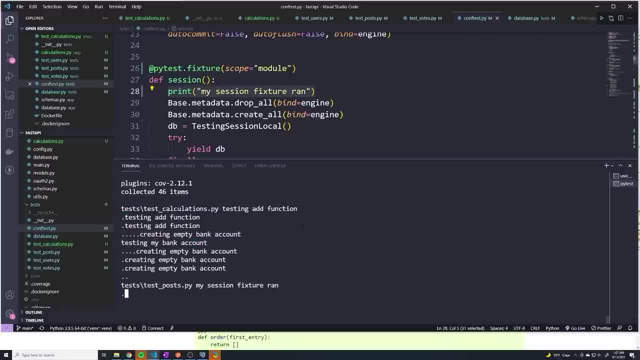 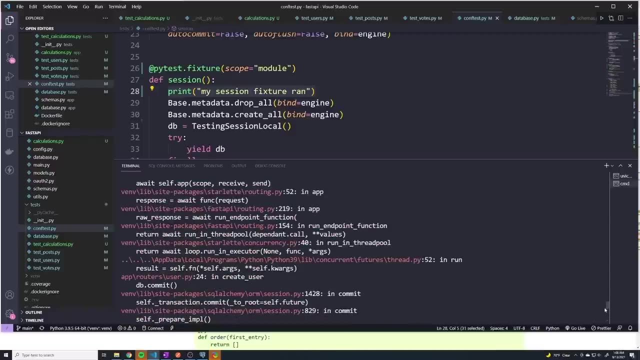 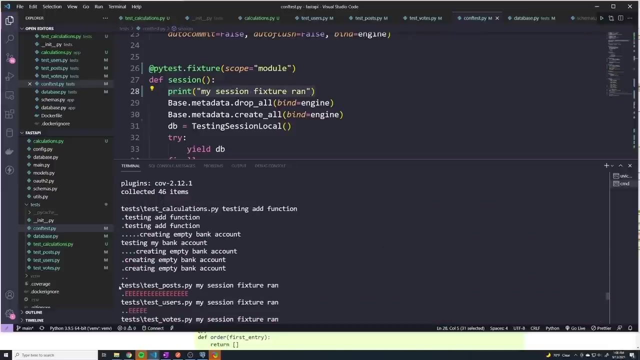 And that's perfectly okay. I want you to notice what's happening. So notice how the print statement ran here. And I had to cancel out of that because usually I end up with a ton of errors and then I lose my data. But you could see that the first module, which is tests, underscore py. we could see that. 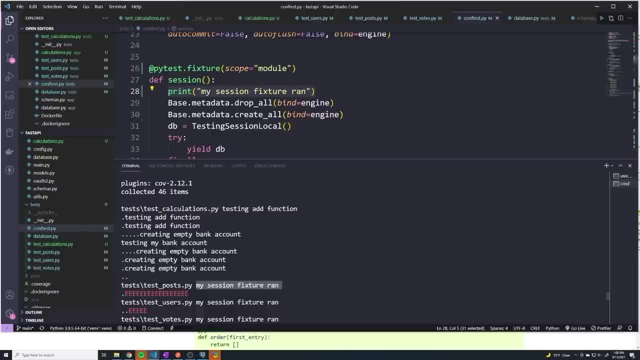 my fixture ran because it's because I told it to run, because one of the tests is requesting it. it runs, then one of the tests runs, And then the next test runs, and then the next test runs. So you could see that this is not printing out per test. 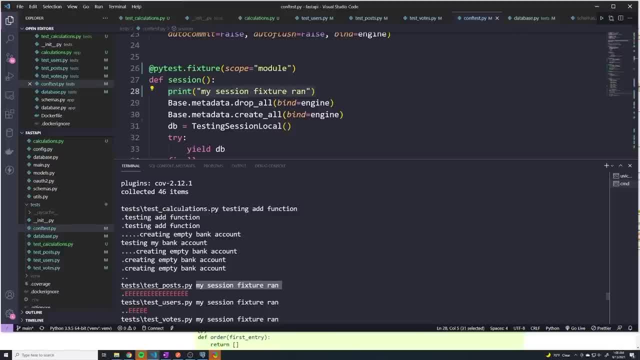 It's only printing out one time per module. So when test underscore post that py ran for the first time and the first test required this specific fixture. it ran once. then it didn't run for any of the other ones. That's why we. 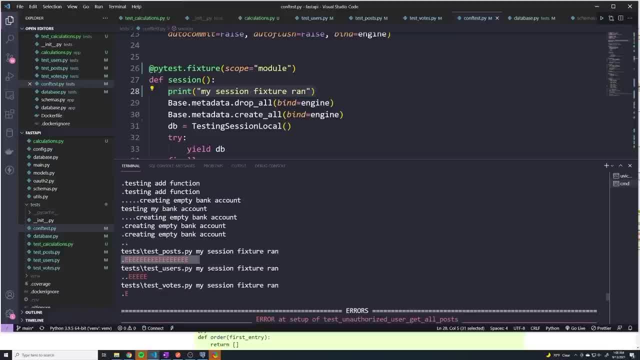 see them all fail And then the next module loads up and we start running tests from there. So we run the fixture just one time And then we don't run it ever again. So you can see seven other. I think it's six or. 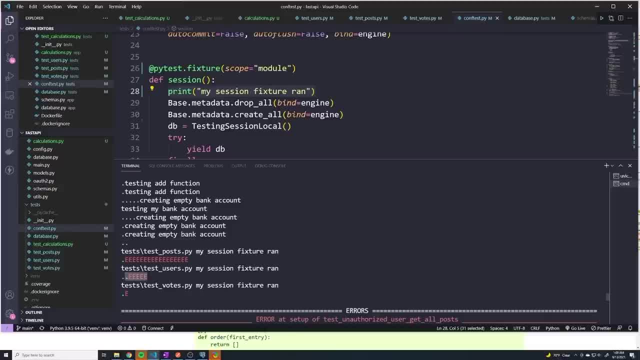 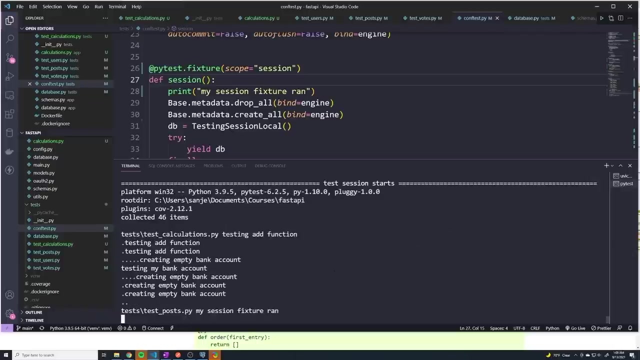 seven other tests ran with no other modules, With the fixture not running any other time. And then we can see the same thing for votes. we can see that my fixture ran just one time, So this means that it's going to run only once per module. We also have session, So if I do, session is going to be even more different. you're going to see it run only one time for my entire testing session. So you can see my fixture ran. it's going to keep going through, which is perfectly fine. And then when we get to the 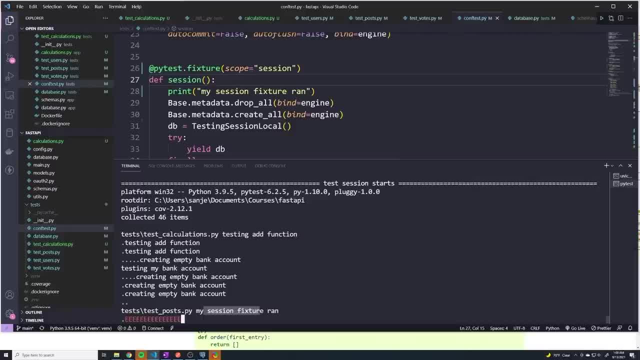 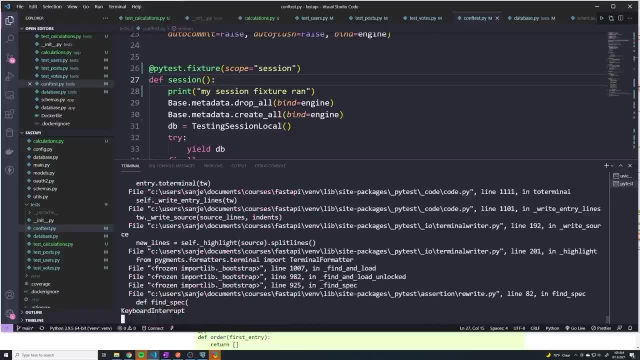 next module. we should see it not run at all, Right, And so you can see it didn't print again. So it's going to go through all of the different modules And I'm going to cancel out of that before I get too many errors. 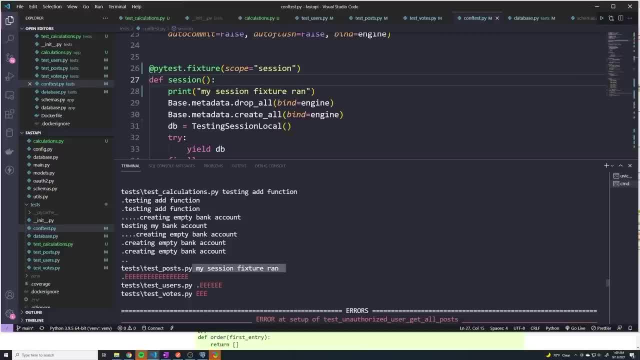 Right, But now it only runs once per entire testing session, So that's when the scope comes into play. So keep in mind, you know, depending on what you're trying to accomplish, you may need to tweak the scopes of your fixtures, depending on what they're supposed to be doing. But for our 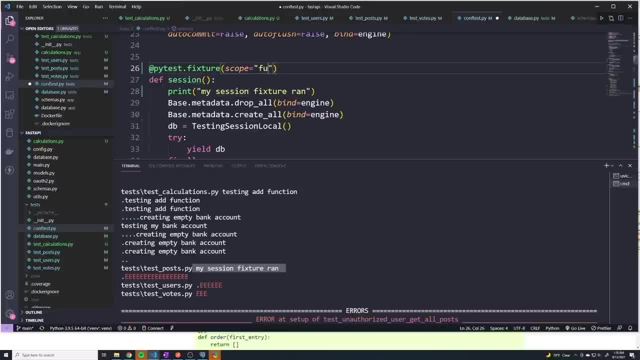 database. we want to keep it set to a function which is the default value, because we want to load up a brand new database by dropping our tables and then creating new ones every single time we run our test. So the default works perfectly fine for us Now to make our login. 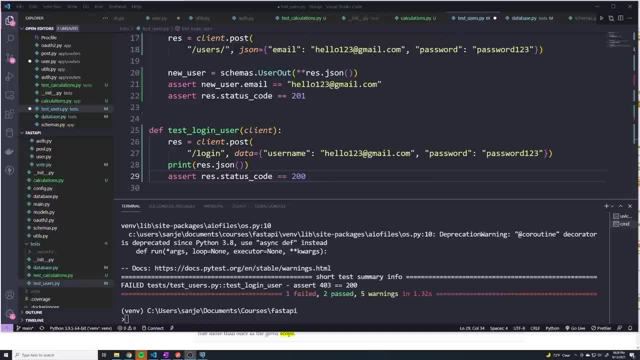 user test independent of any other test, so it's not reliant on a specific order or setting the fixtures to be of a specific scope. What we want to do is, before our login user test runs, I want to actually go in, define a function that'll get called, that'll actually create a brand new user. 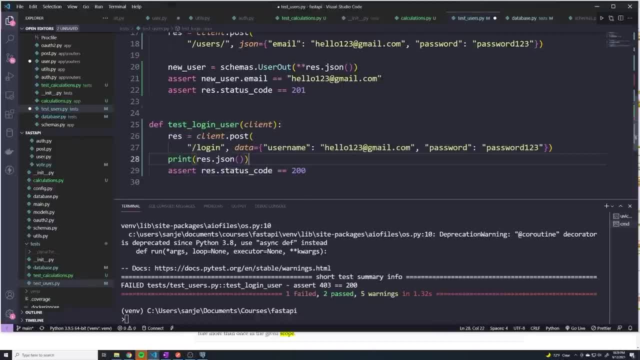 so that we can actually test the login user out. And so you know, as soon as I said the words I want to run a function before a test runs, the first thing that should click in your head is: you want to run a fixture or you want to create a new fixture. 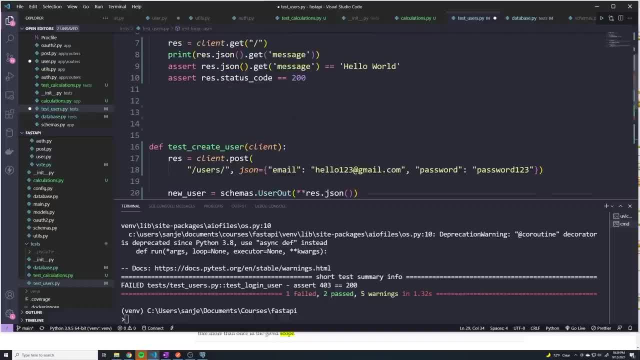 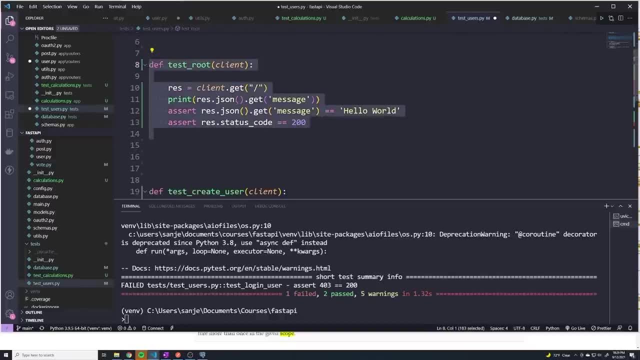 So we can actually create a fixture. that will create a test user for us. So up here at the top of this file, let's create a new fixture And I'm actually going to delete this test. we don't actually need it anymore. It's just taking up space, or I can at least comment it out, I guess, And I'm going to. 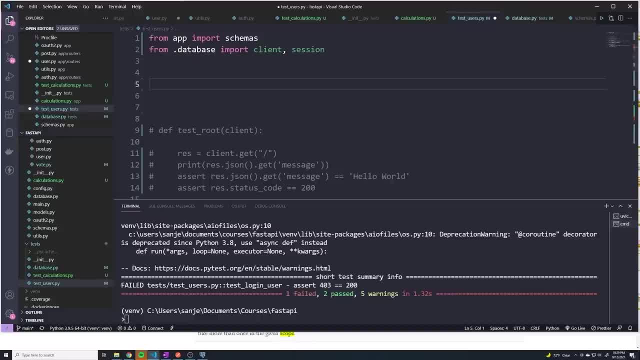 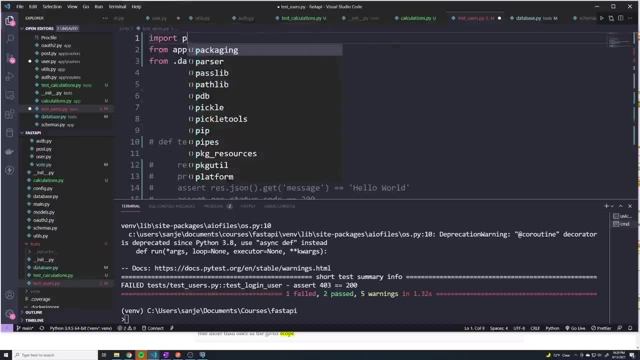 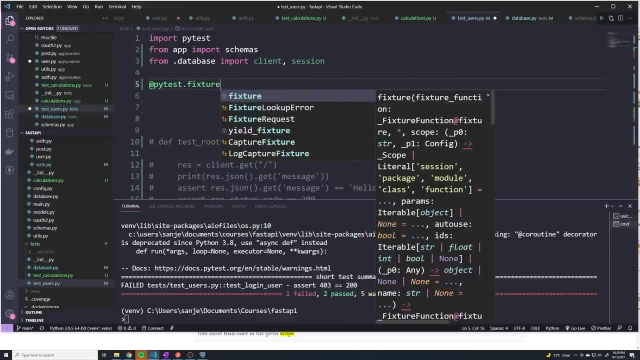 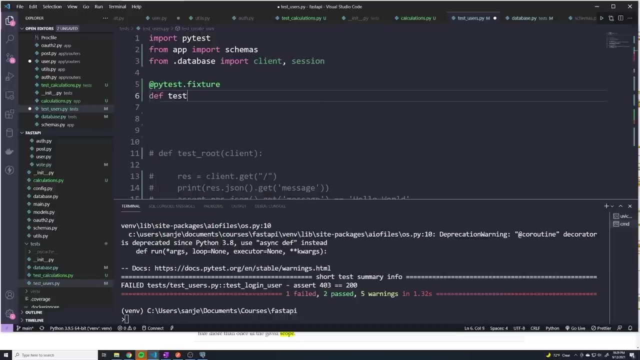 create a fixture here And we have to import pi test, we'll say from whoops, import pi test. And we'll say at pi test dot fixture And I'm going to call this test user. So it's gonna be responsible for creating a test user. 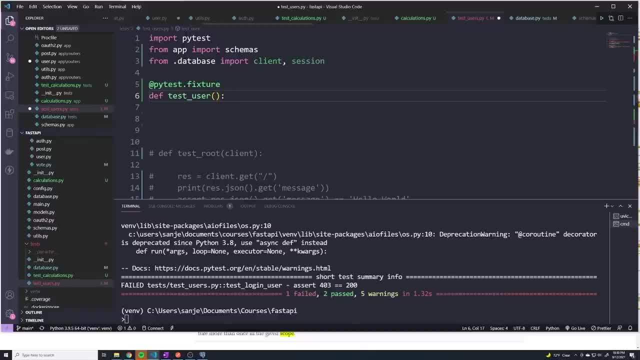 And this is actually going to make a call to our create user route. So we actually need access to client so that we can actually make that request, And there's two different ways of doing this. right, we could just have access to the session object. we can have access to the session object. 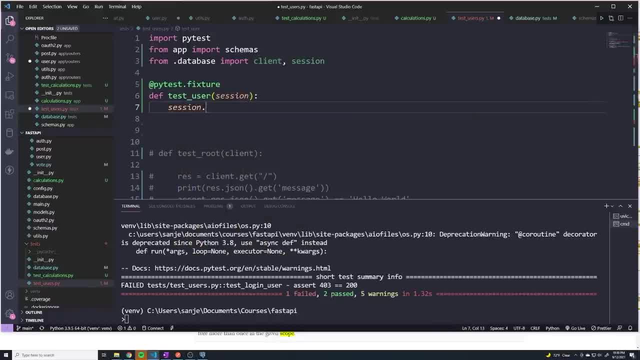 and we can just, you know, session dot. you know, I think what is it actually? no, it would be like models dot user and then passing the data for a test user and then create it directly with the database, Or we could just make a call to our API. 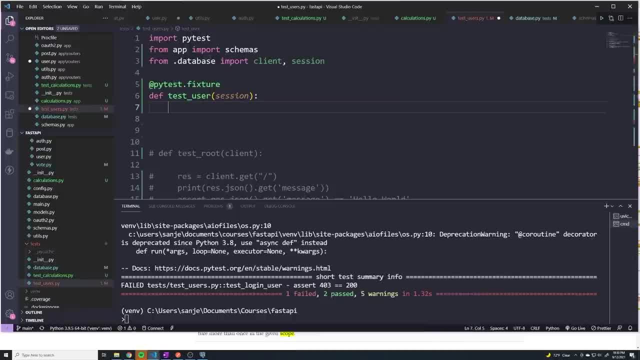 And actually have it run through that. So I'm going to do that because it's a little bit simpler for now, But I'm going to define a, a dictionary with the data that I'm going to use for my users. So I'm going to have the email And actually it's going to be a little bit easier if I just paste. 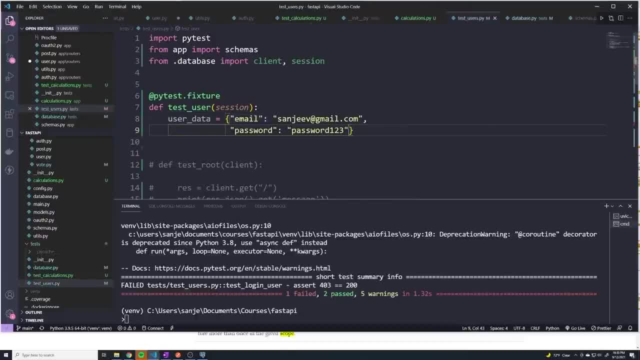 this in, So we have the email set to something and then the password set to something, And I'm going to change this back to client And now I can say res equals client dot post and we'll send it to users And then the data for the new user can just be user underscore data And just 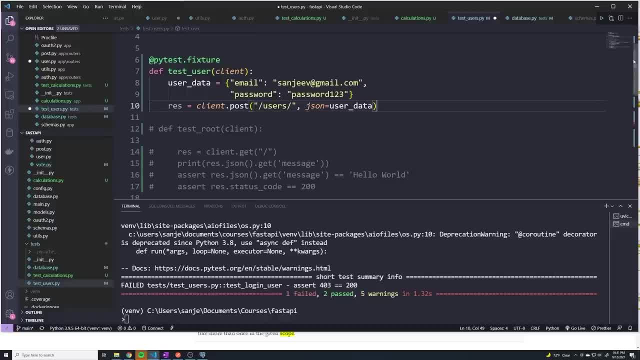 kind of like what we've done here. we can you know, just to make sure that this did an error out, we can do an assert And just say you know, res dot status code equals equals 201.. If that's good, I think it's safe to assume we. 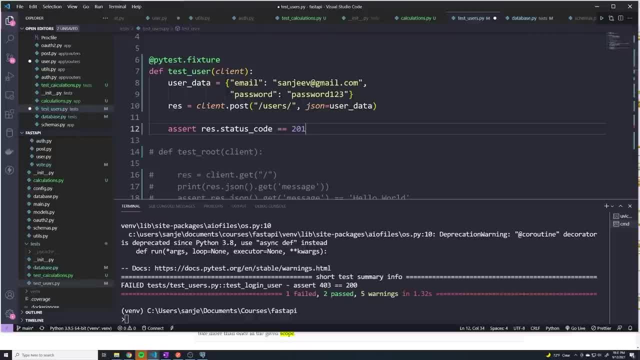 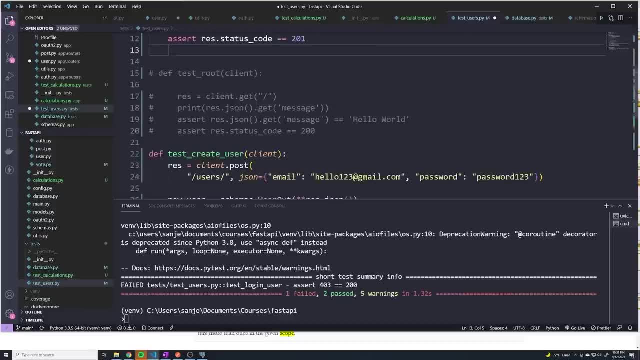 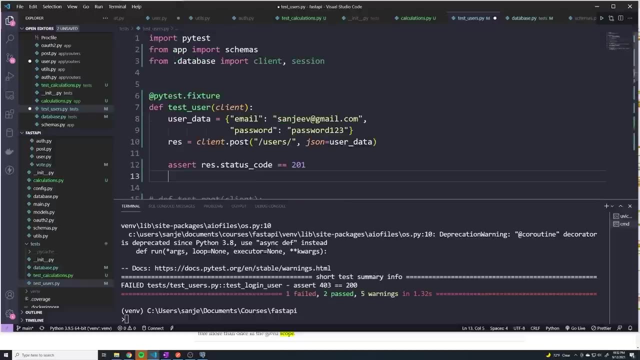 didn't run into any errors on on the back end. But then what I want to do is, not only do I want to create the test user, I want to actually return the information about the user so that this login user will have the correct data to send when he tries to log in. That way, if we ever change this, 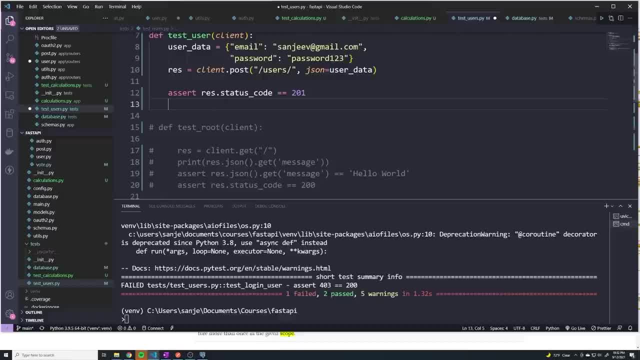 data. we should automatically update this data. So what are we going to return? Well, we have access to what is it called to res dot JSON And if I print that out, we can just quickly take a look at what that looks like. And for now, I'm just going to return. 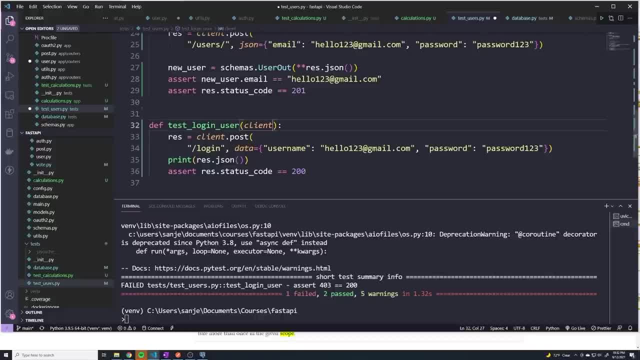 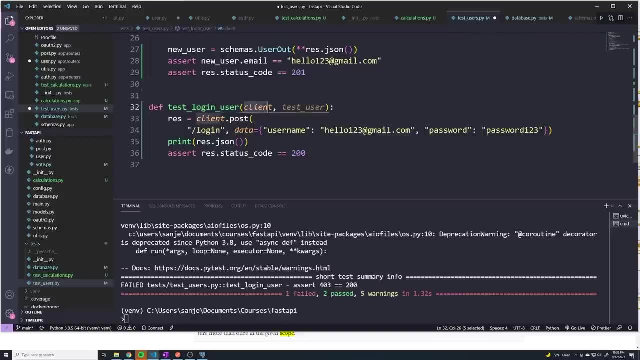 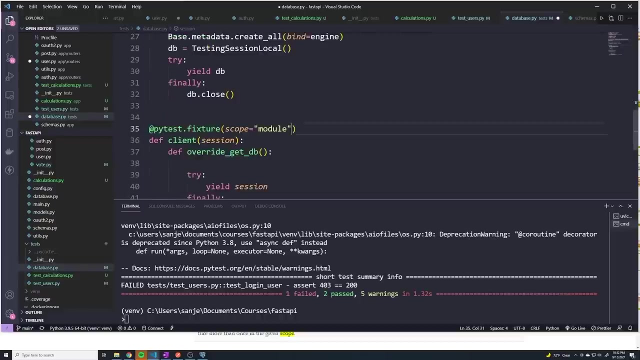 nothing. I guess that's fine. I'll just return nothing. And here I'm going to change this to be: I'm going to pass in the test user, So that also runs. And so now this login user is dependent on two different fixtures: client and test user. And before we do anything else, let's make sure we clean up the scope. we don't need these to be that to that anymore. 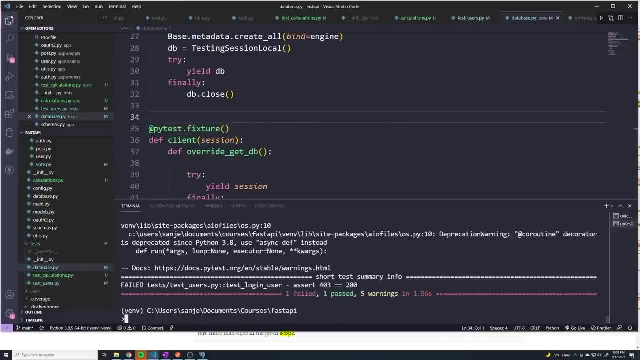 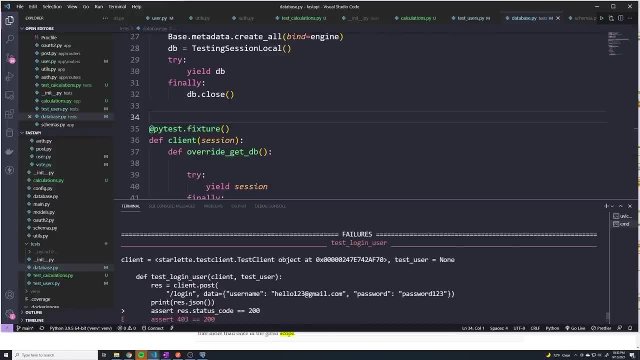 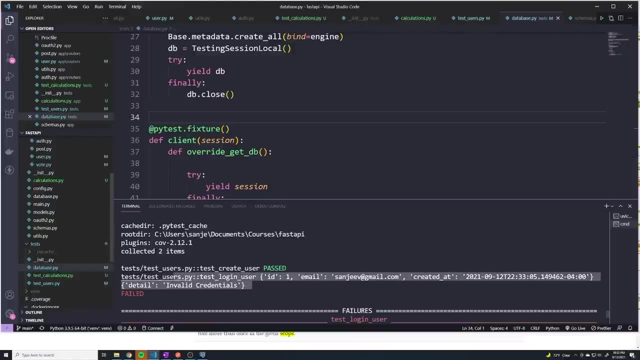 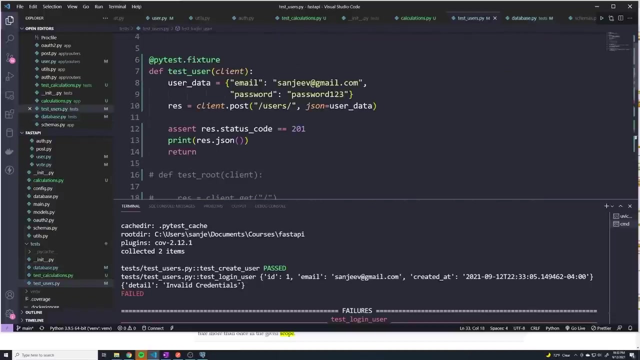 And if we run our tests, all right, the data we get back. we get the username- I'm sorry, that's not what I want. this print, we get the ID, the email and the created at on. So what we'll do is I'm going to actually take this dictionary And I'm going to pass in the password as well, Because when I actually go to log in the user, I need to make sure that he has access to what my password is, But that doesn't get returned in the response. So what we have to do is we'll have to add a new field, so I'll say new underscore. 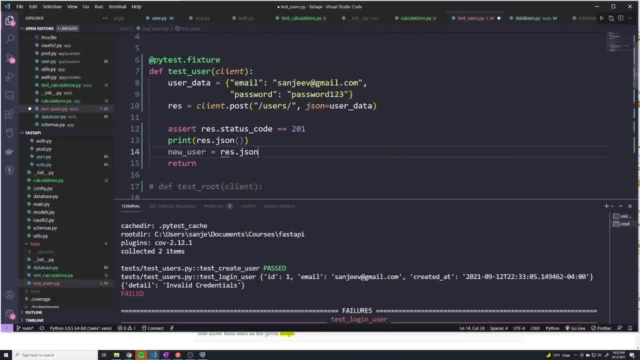 user equals, you know, res dot JSON. So we get that dictionary And then we'll say new underscore user, we'll add in a new field new key called password And I'll pass in user underscore data, which is this dictionary. 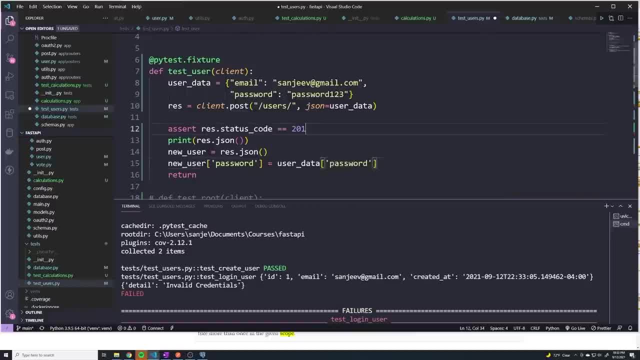 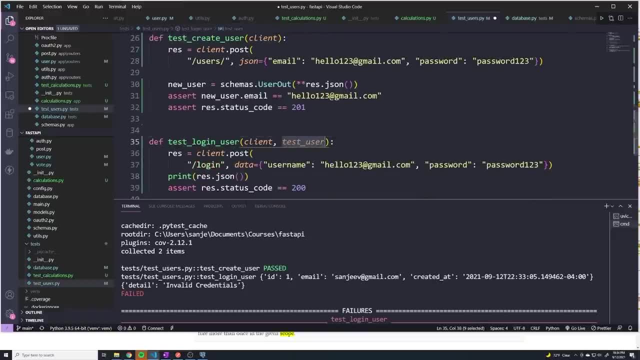 up here And we'll grab the password from here, And what I'm going to do is then return new underscore user. And so anytime someone calls test user, or anytime we have a test that's dependent on that, it's going to run this function. it's going to return the new. 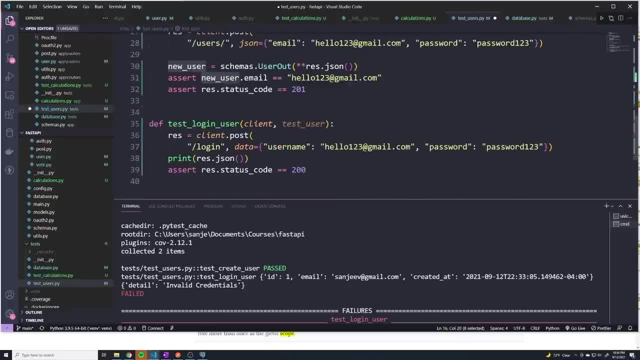 user. And so now that we have the new user, what we can do is I can say the username is test underscore user And we'll grab the email key and then the password will be test underscore user And this will be password. Okay, and so that way, if I ever change the 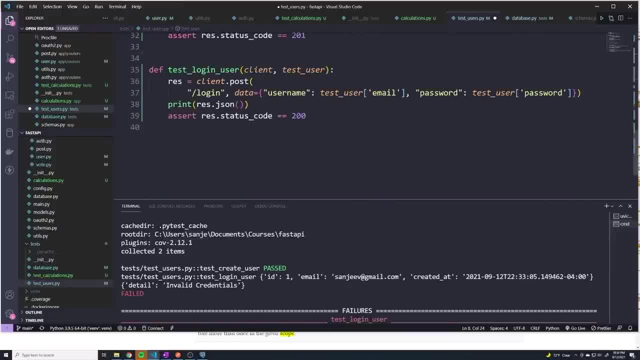 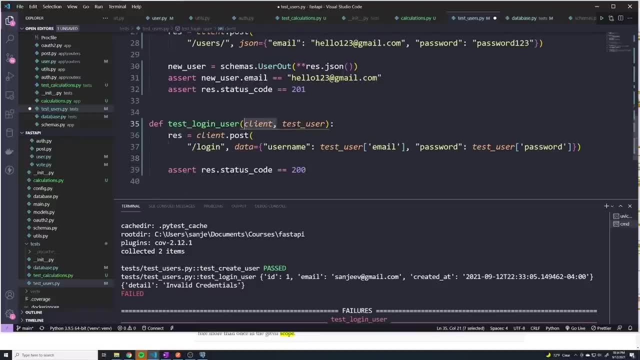 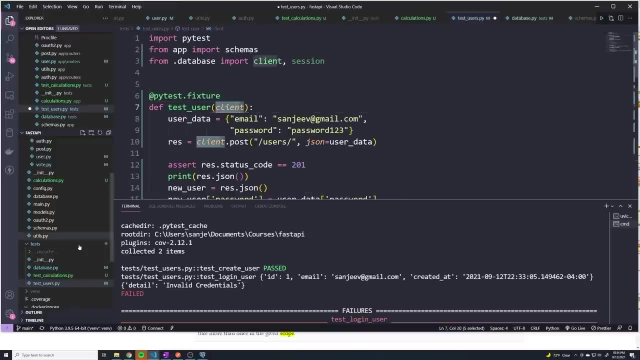 password up here. it's going to automatically get updated down here, So we don't ever have to worry about that. And one thing to note is that, technically, if I deleted this and just call test user right, Victżein, a test user would technically call client and that would go all the way back. 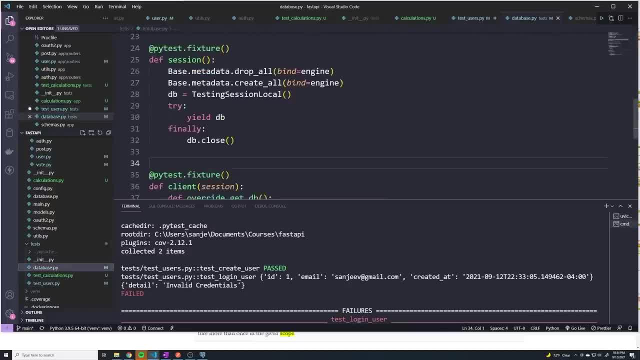 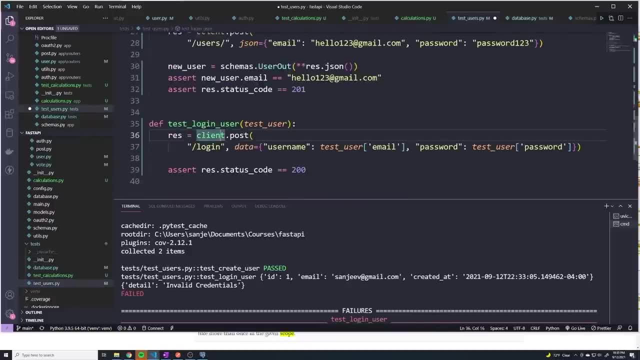 here And then client would technically call session, So it would call all of these functions automatically for us. However, the one issue is that in this test we still need to make a call with clients, So we still have to pass in the client objects that that we can make. 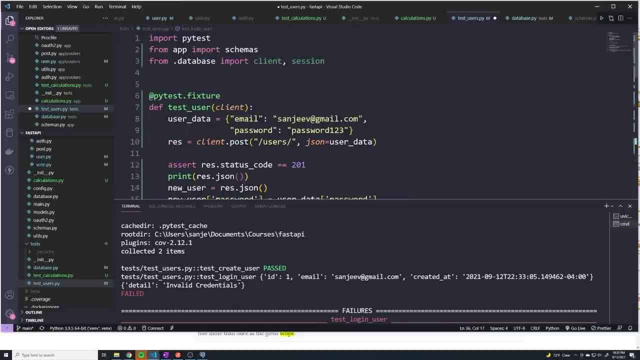 use of it. But I did want to highlight that because this fixtures dependent on client, it will run whatever code is in the client fixture And because client is dependent on session, it will run whatever code is there within the session. So it's all done automatically for 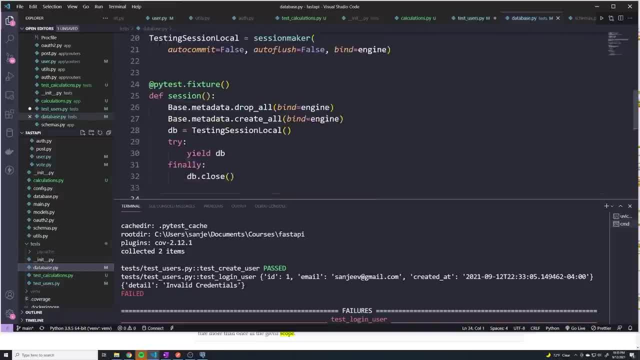 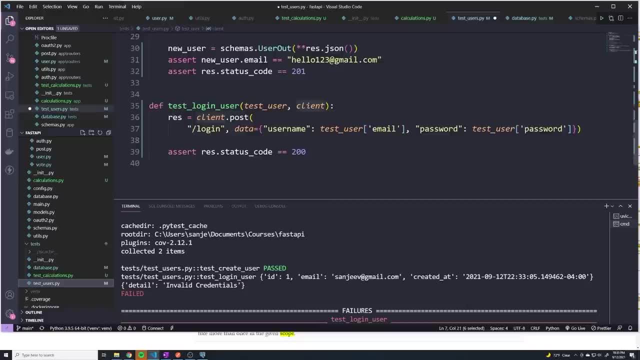 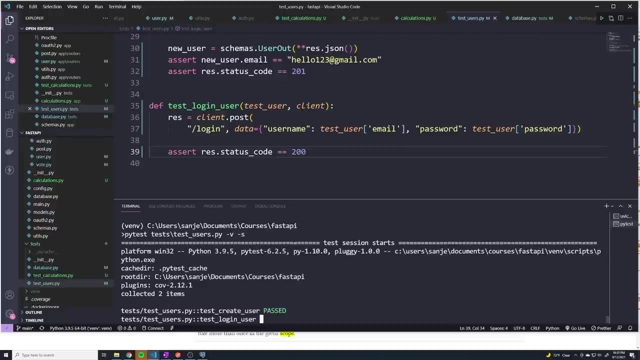 us Right. So the order once again is going to be: we'll run session first, we'll then run client and then we'll run this test user. So let's test this out now. Hopefully this works And it passed Perfect. Look at that, guys. we were now successfully able. 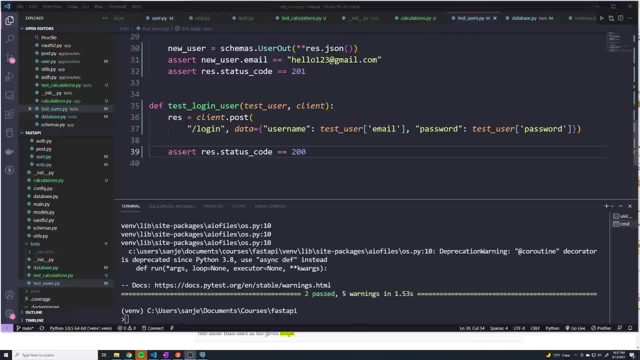 to log in a user. So that's cool and all. but I want to do a little bit more validation for the login user route, Just to make sure that you know we got a token, the token is valid, And just do a few extra checks. So, just like we did with the test create user- we have we can take use or we. 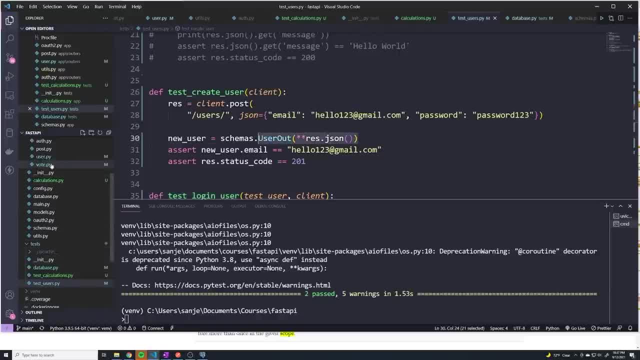 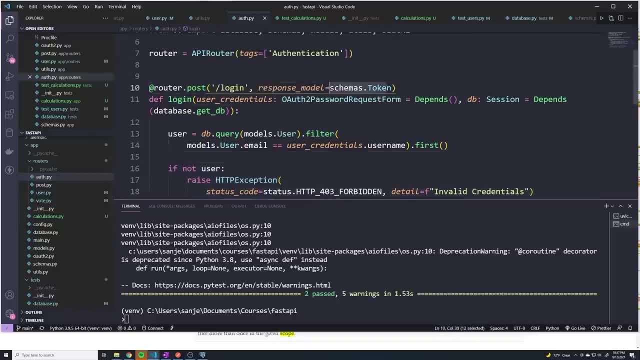 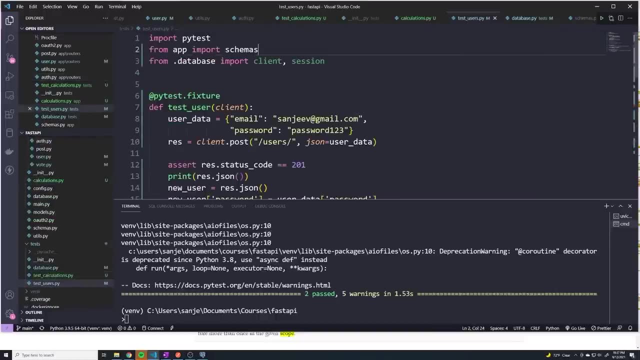 can make use of the pydantic model that we use for the response. So if I go into my authpy under routers and we can see for the login the response model set to a schema token, So let's import token inside our test userspy. So here schemas: we already have access to schemas And so I can say: 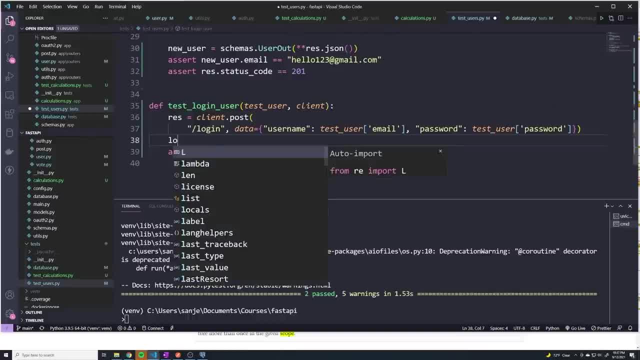 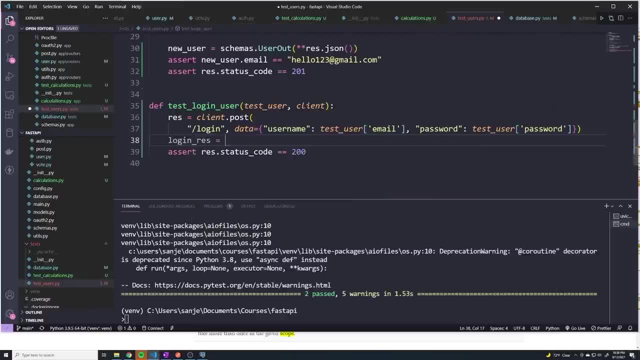 token, or what should I call this? I'll just call this login res, which equals, and then we'll call in schemas dot. I think it was a token. was a token or token data? I think it was token. Well, let's just double check. 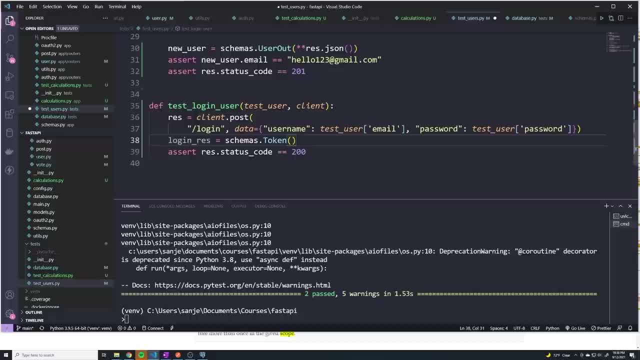 It's token, perfect, Okay, so token. and then what we're going to do is we're going to spread res dot, JSON, All right, so that's going to perform a little bit of validation, Right? And then, when we get a token, I want to actually validate it. 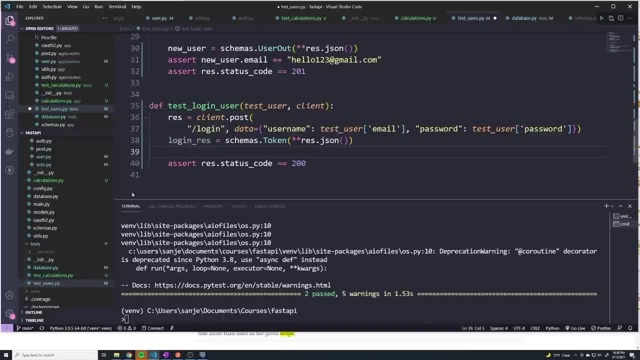 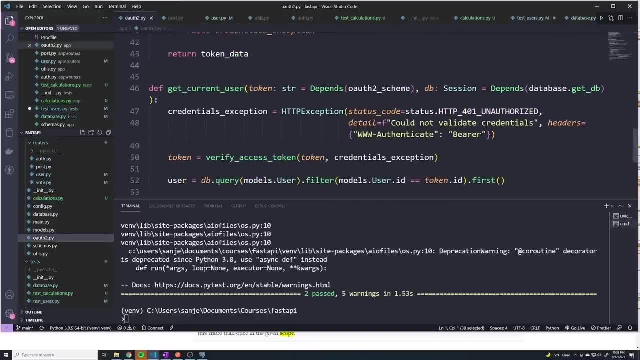 So how exactly do we validate it? but we want to decode the token, And so all of the logic that I'm going to implement here is essentially the logic that we use within our OAuth 2 py file. So when we want to get the user, 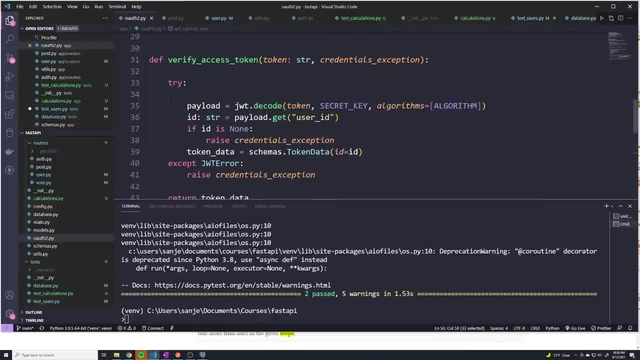 we want to verify the access token is valid. So how do we do that? the all of the logic is right here. So we're going to decode the token And we're going to make sure that the user ID is within that token, And that's all I'm really going to do at that point. So I will copy this. 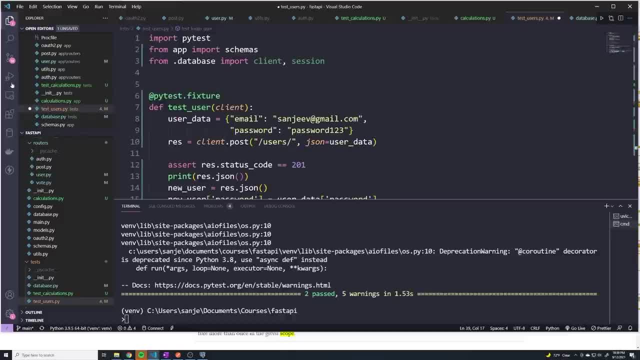 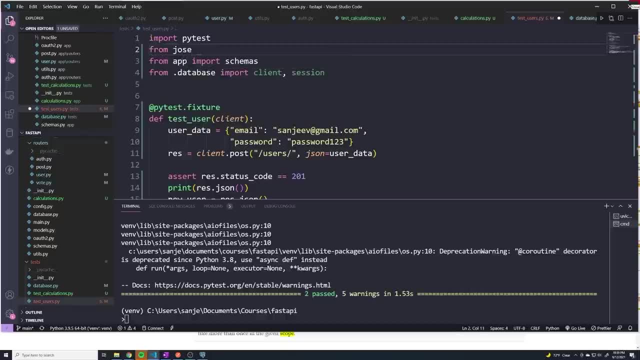 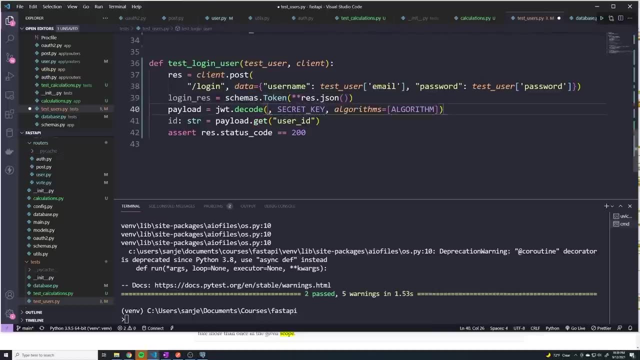 And we have to import JWT from, so from- I don't know if it's Jose or Josie who knows- So import JWT, And what will decode is going to be in the login underscore, res, under the access token property, And then we have to pass in the secret key as well as the algorithm. So 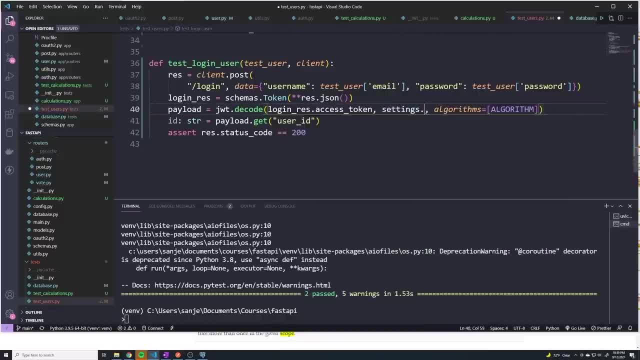 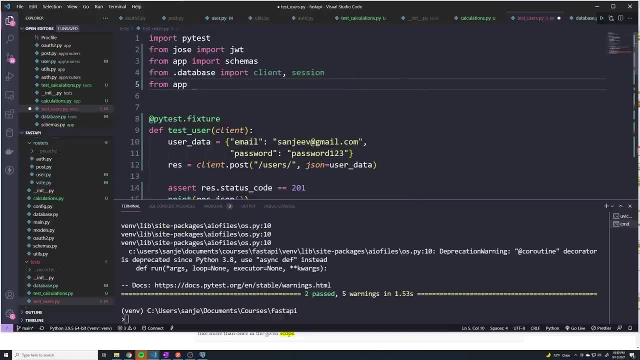 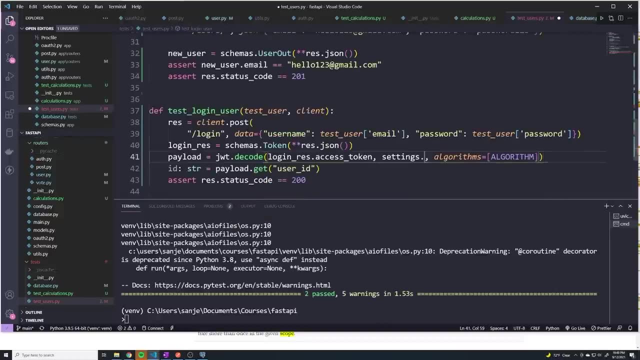 the secret key can be accessed with settings dot. well, I have to import my fig. So I'll say from app dot config, import settings. And now we have access to our environment variable. So I'll do settings dot secret key. And then the same thing goes for the algorithm. So I'll set this to settings dot. 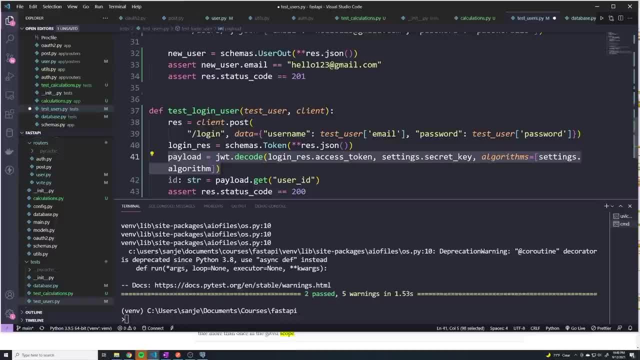 algorithm So we're able to deload it, decode it, And then I'll remove this check. I'll just say: ID equals payload, dot get user ID. And so once we get the user ID from the token, what we can do now is I can just assert. 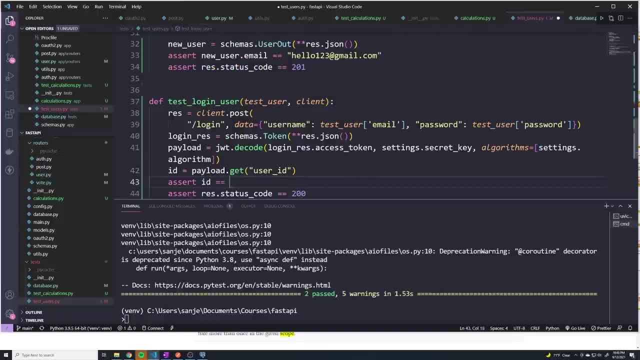 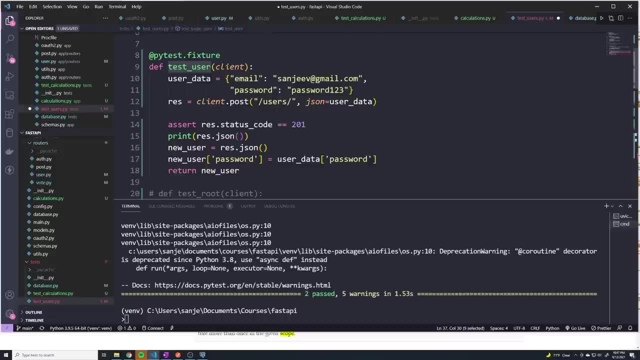 does ID equal, equal, And then is it going to match the ID of test user? So if we take a look at what test user was, that's coming from this fixture And so it's going to return. Oh, it looks like I did not. No, no, it should be in there. So, since we grabbed the response, the ID should be. 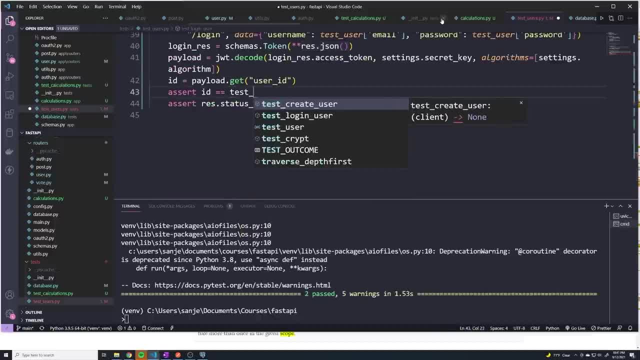 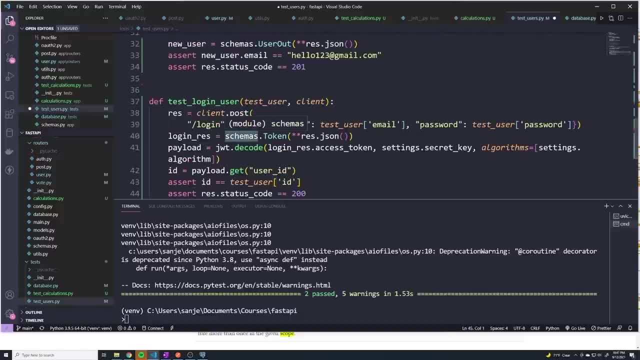 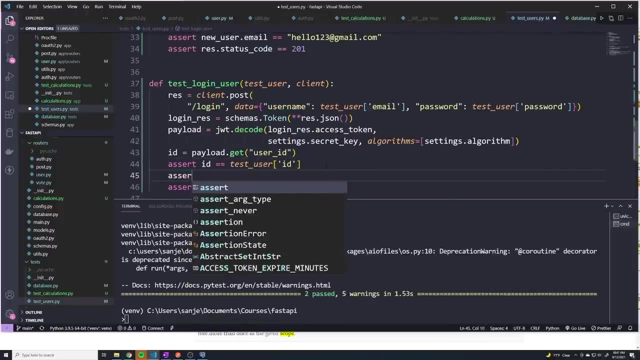 there. So we can just call this test underscore user and then we can just call ID. So I think that's a little bit more of a valid check, because it's actually decoding the token just to make sure we didn't break anything there. And one more thing: We can assert login underscore res dot token. 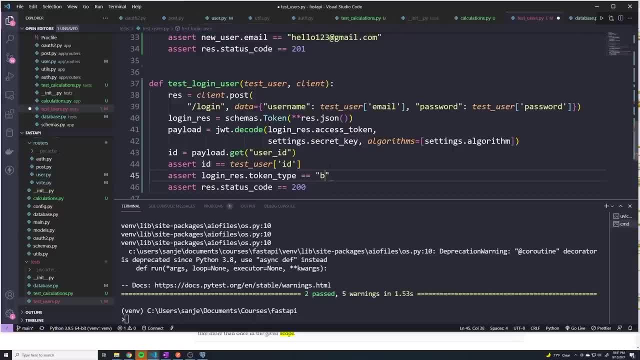 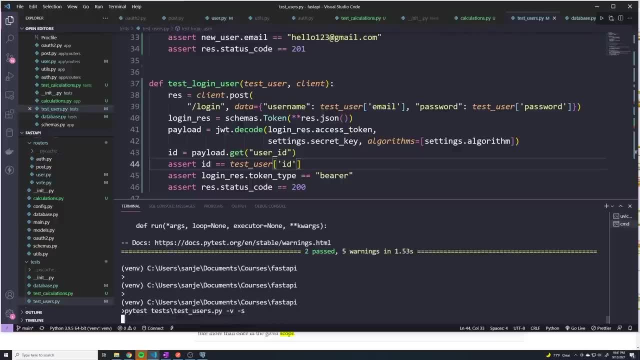 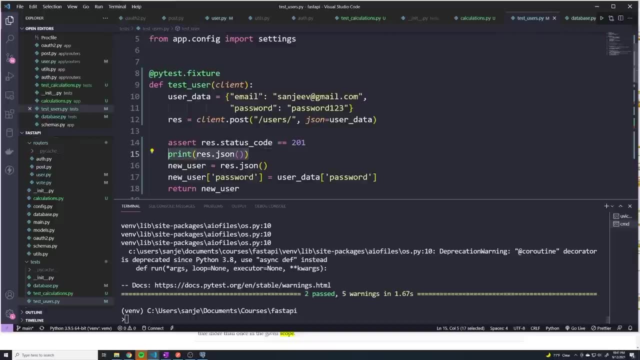 type, So this should be set to bearer. All right, so let's test that out now, And everything worked, I think I've got one random print statement that I don't want, so I'll just remove that, And we have now successfully completed our login user test. 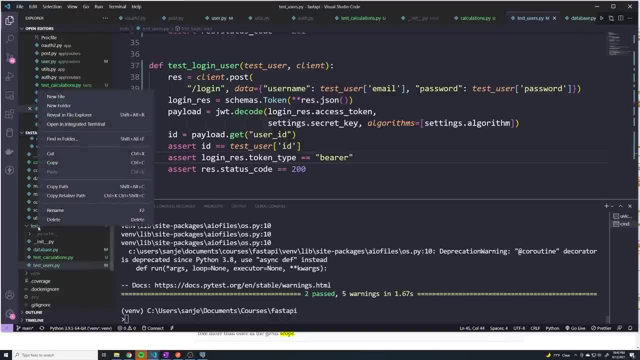 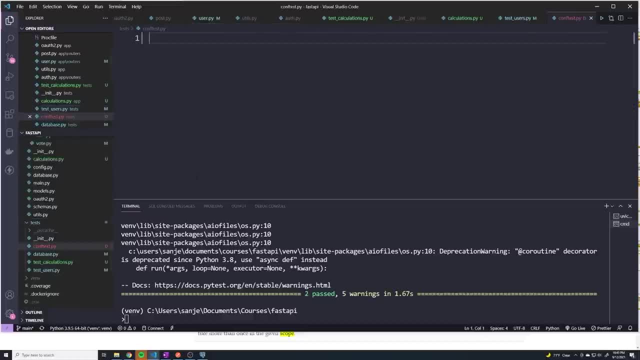 Okay, guys. so before we actually create any more new tests, what I want to do is I want to create a special file under our test directory called contestpy. So this is a special file that pytest uses And it allows us to define fixtures in here. 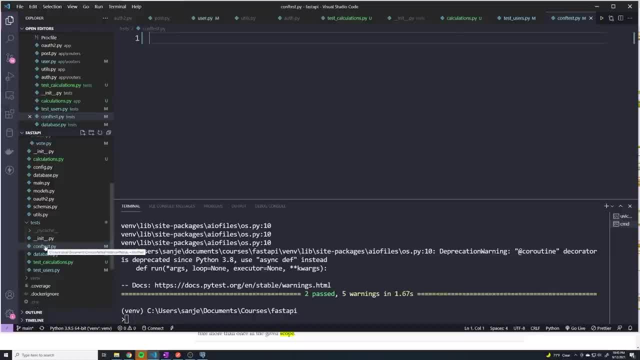 and any fixtures you define in this file will automatically be accessible to any of our tests within this package. So it's package specific. So anything within the test package, even sub packages, will automatically have access to any of these fixtures. The reason I want to do this is I 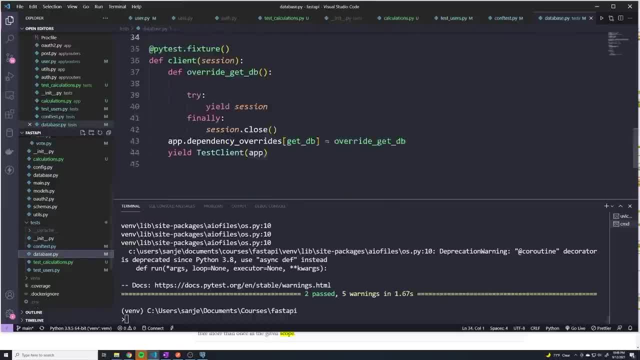 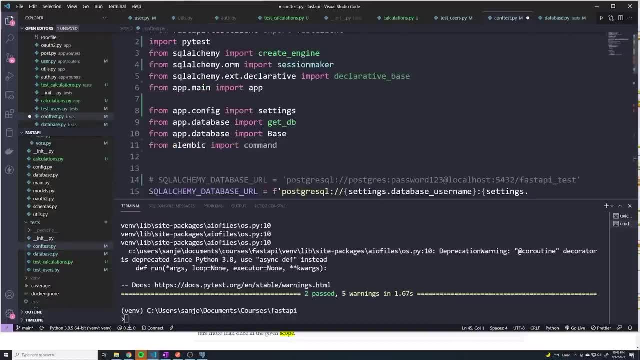 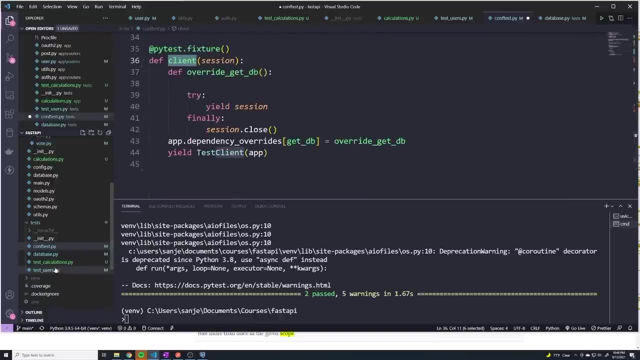 want to take all of our database code essentially, or our database fixtures, and I want to copy all of it And I want to move it to contest. And so by moving it to contest, this fixture, the session fixture as well as the client fixture, will all be accessible to you know. test calculations. 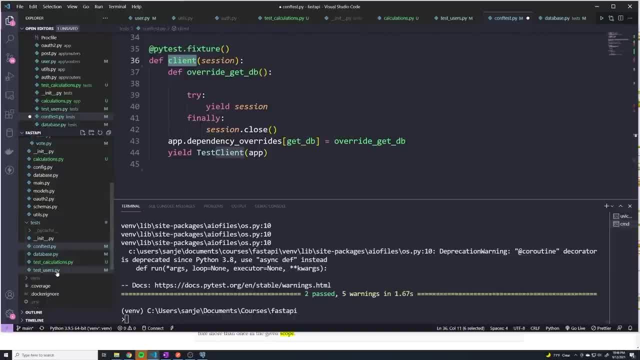 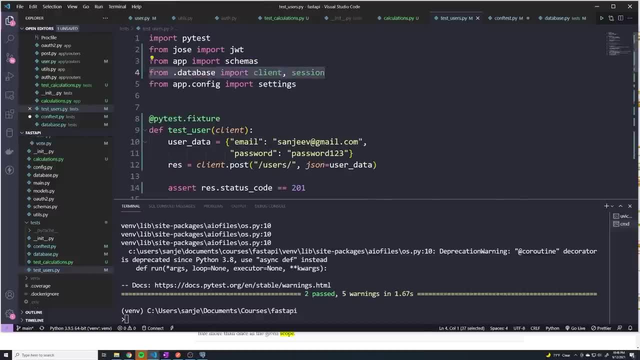 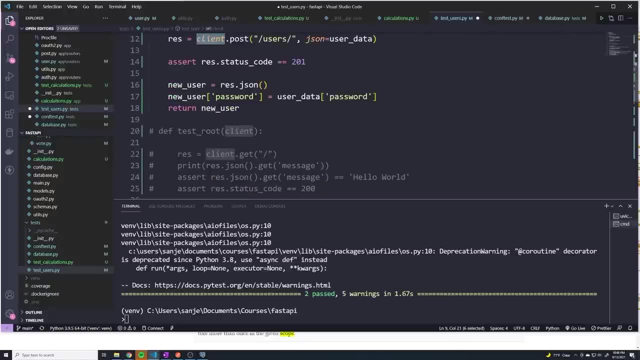 test users, any other test files within the test folder automatically, And so now I don't actually have to import anything, So I don't need to import from contest. it'll automatically do that, It'll automatically have access to client and it automatically have access to session. And what I'm actually going to do is I'm going to move. 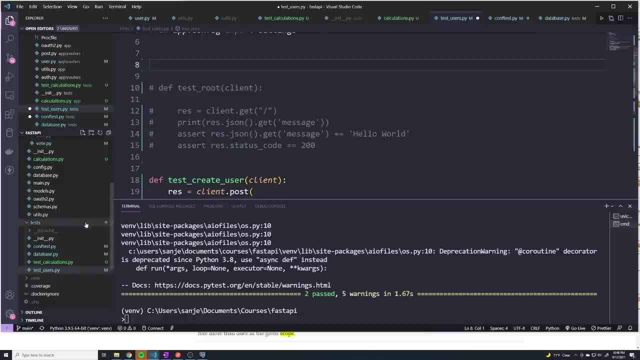 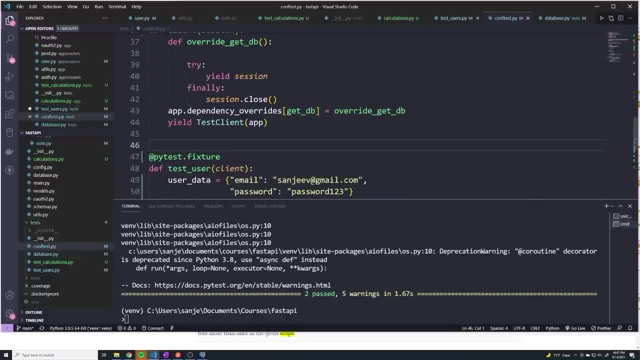 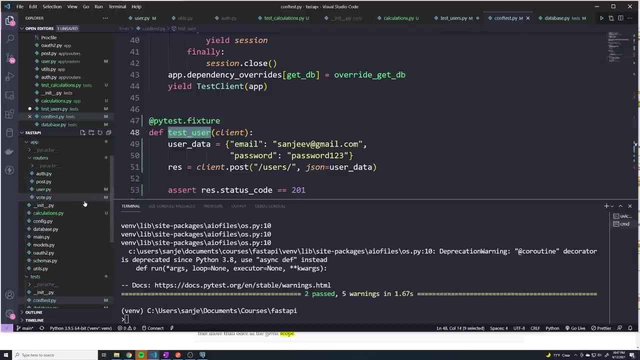 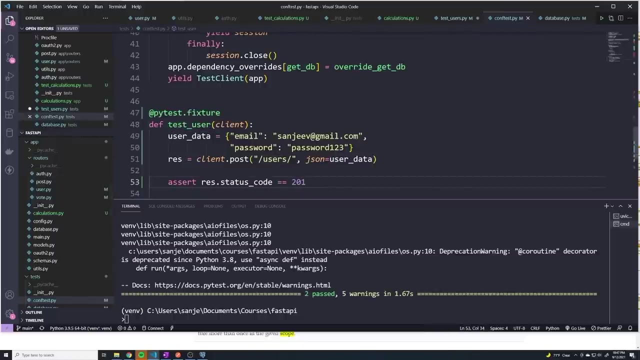 this test user to contest as well. And so that way, because I imagine that even for other modules that I create, you know, especially like for voting and a few and creating posts, they're going to need test users as well. So it makes sense to put this in this contest So everyone's 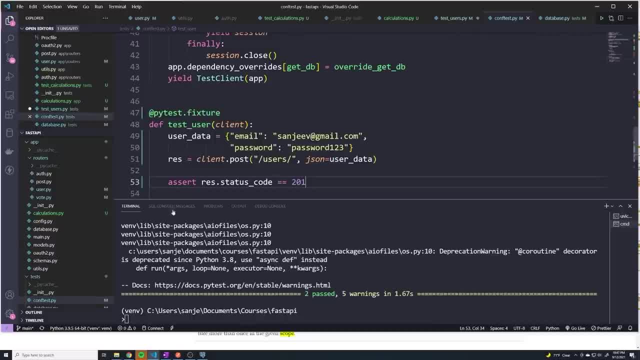 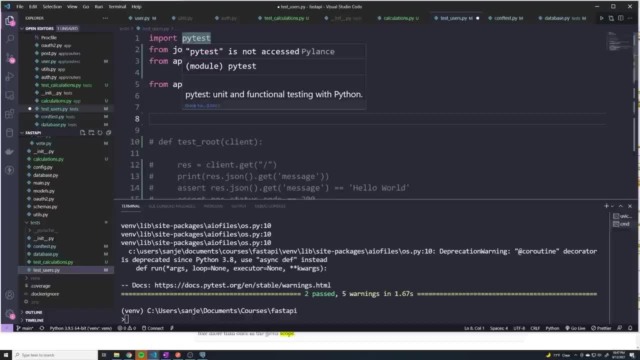 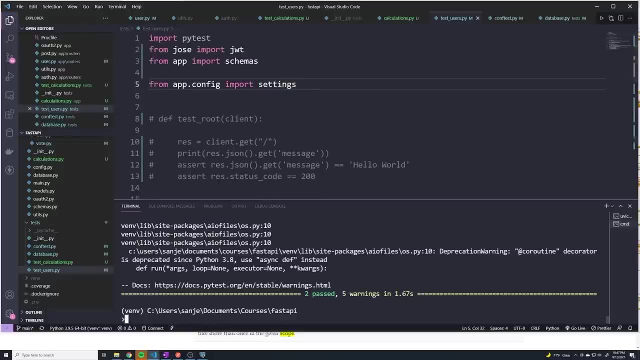 going to have access to it And I don't have to go around constantly importing things around like that. And now, within our test users, I should be able to leave everything else And you'll see that we're not importing client or test user anywhere here. But when I run this, we should see no issues. 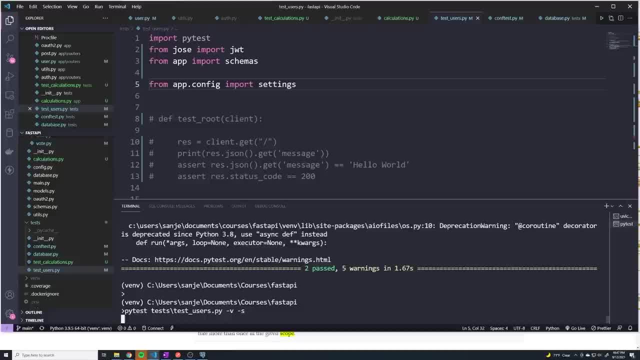 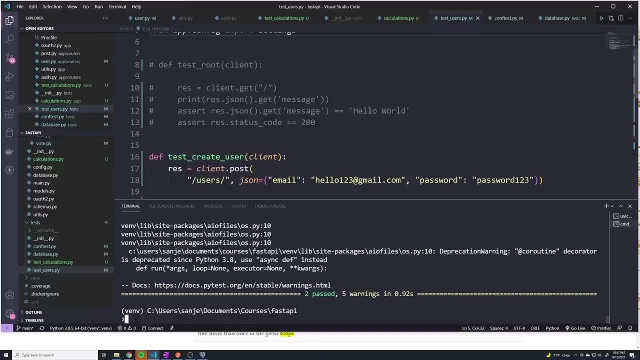 So let's give this a try And you can see all of our tests passed with absolutely no issues, Because we are importing those From the contest file And keep in mind, you know, let's say I created a new package. I'll call this. 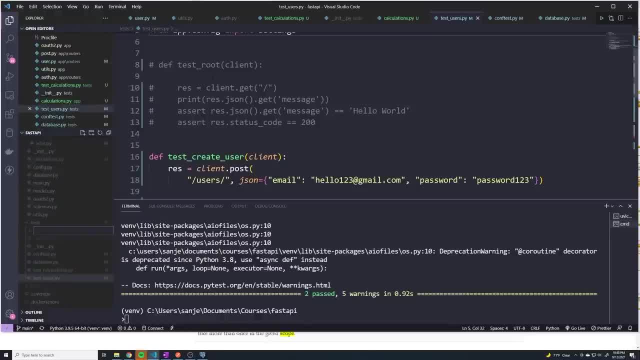 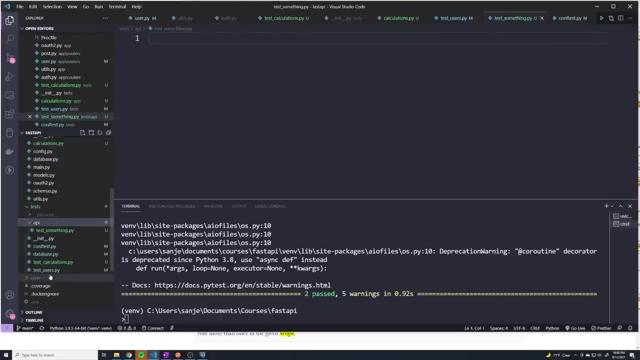 whatever. how about API or something? it doesn't really matter what I call it, And I've got a whole bunch of tests in here. you know, test underscore something, that py, Because this package is still within the test package. it'll have access to all of the mod, all of the fixtures in the contest py. 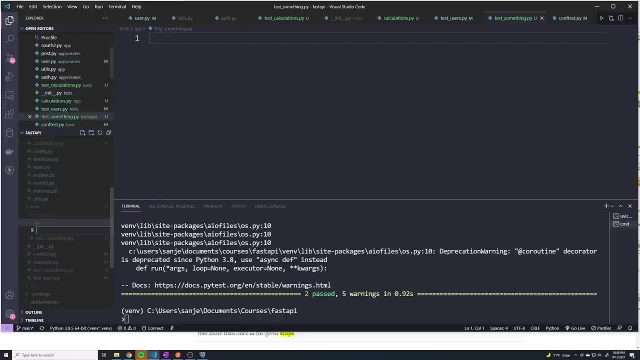 But within a package I can also create a new contest. So I can make a new contest that py down here as well, And when I do it within this package, then test users doesn't have access to that one, But anything within the API package will have access to the fixtures in the API folder as well. 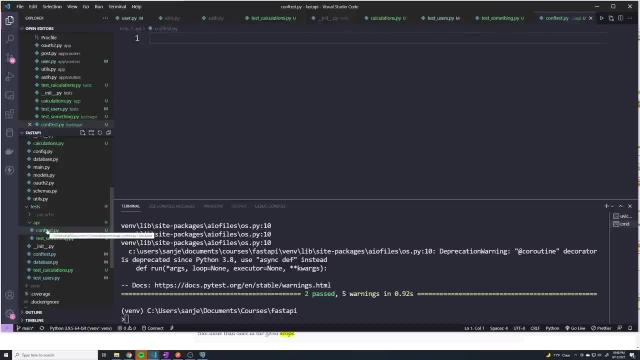 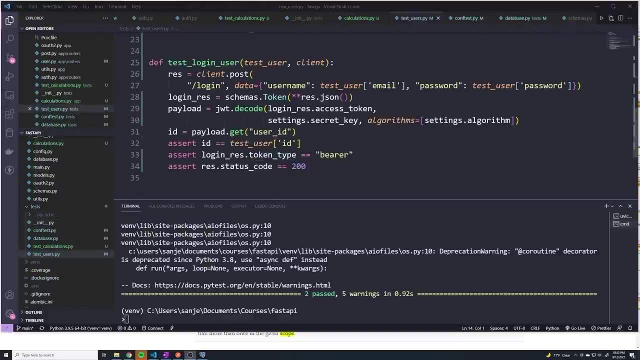 So contest is package specific. So every directory you create you can create a separate contest file so that you can essentially scope fixtures, or you can make it so that fixtures are automatically imported into certain parts of your tests And not others. But we'll delete that because I don't actually need that. Alright, so we've finished. 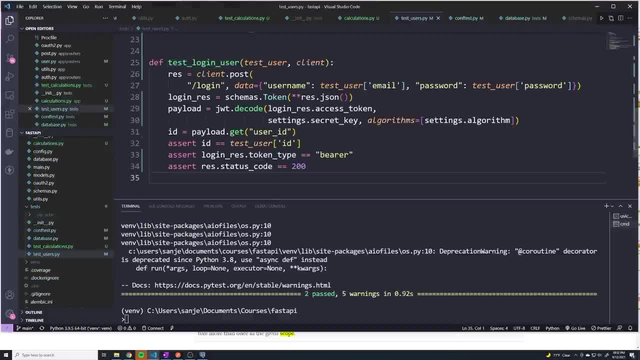 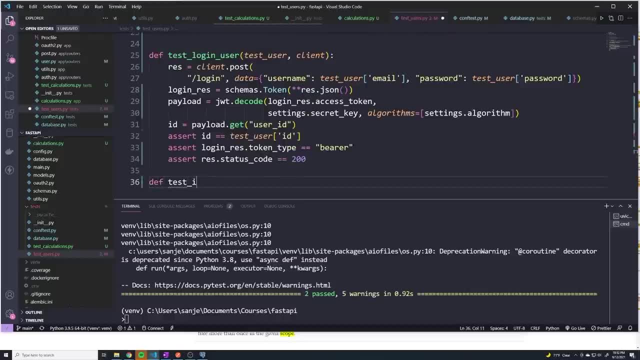 our successful login user test. The next thing we want to test is for a failed login, So I'll do the same thing. I'll call this about test incorrect login And once again, a few things need to happen. let's we want the test user, so that a test user gets created So we can try to log in with his. 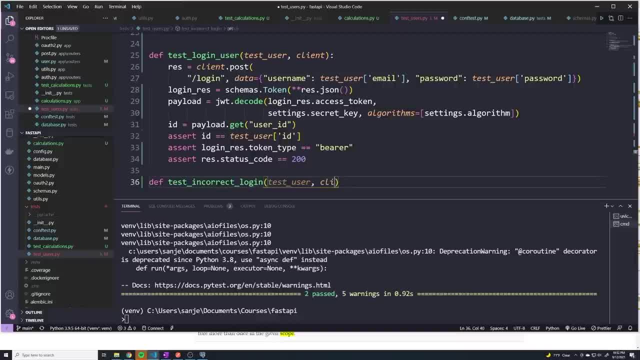 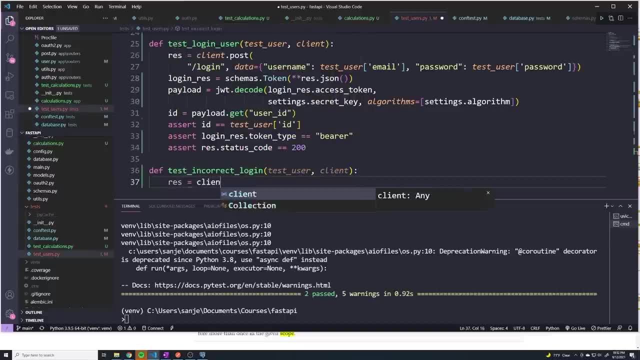 credentials, or a least with the wrong credentials this time. And we do need access to client, just because we're going to be making a request, And here I'll say res equals client dot post And we'll say login And for the login data We'll say data equals, and then we'll do a dictionary here, the username. We can. 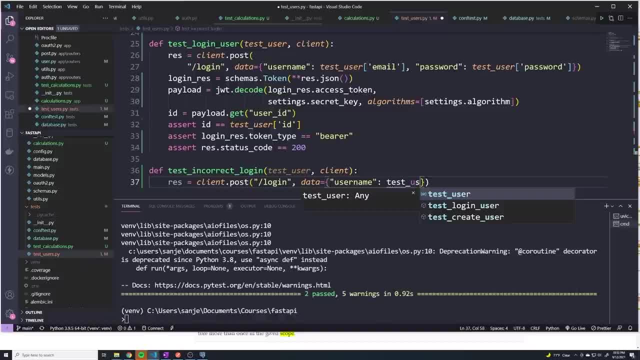 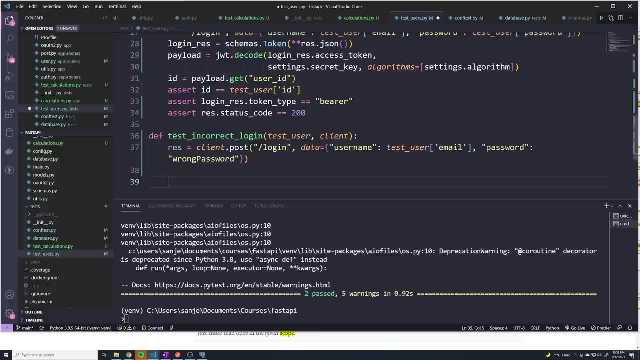 use in this case, test, underscore user Email And then for the password, We can just- I mean we can just- give it any arbitrary password. we'll just say wrong password. So we know that's the wrong password. And so when a user enters in, 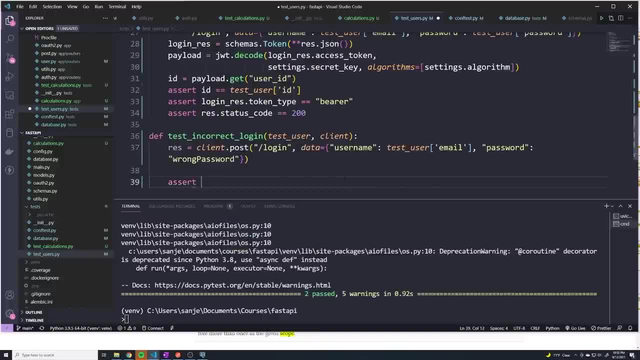 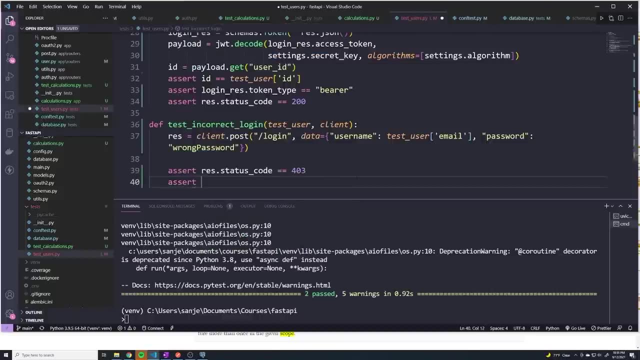 the wrong credentials, we should get a 403.. So we'll say: assert res: dot. status code equals: equals 403.. And in the response it should tell us that we have invalid credentials. So I'll say: assert response, dot. JSON. I will convert. 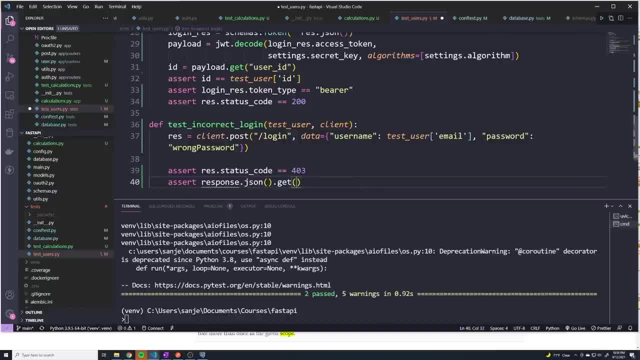 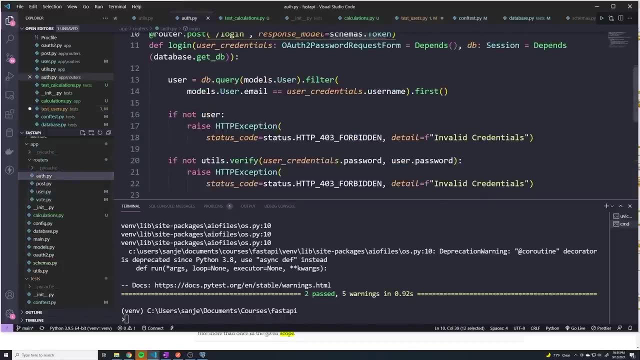 it to JSON, we will get the detail property And that should equal invalid credentials. make sure you get the capitalization correct, because it's going to do an exact comparison And just to confirm if that's what the capitalization looks like, it should be invalid credentials, So just copy it. 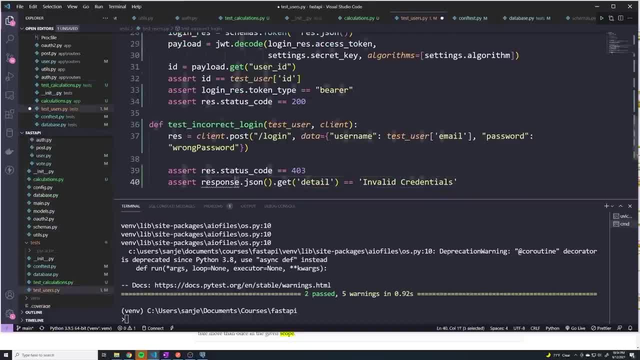 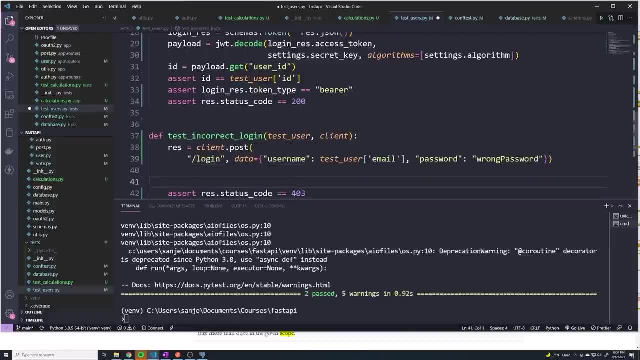 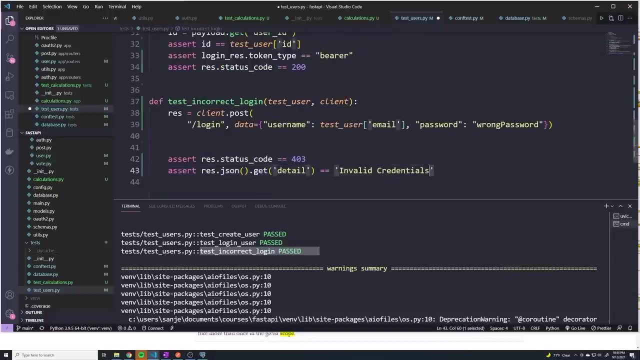 directly from here, And this should be res, Not response. Let's try this out. All right, and the incorrect login worked. Perfect, So that means we did get a receipt, we did receive a 403.. And we did receive the message invalid. 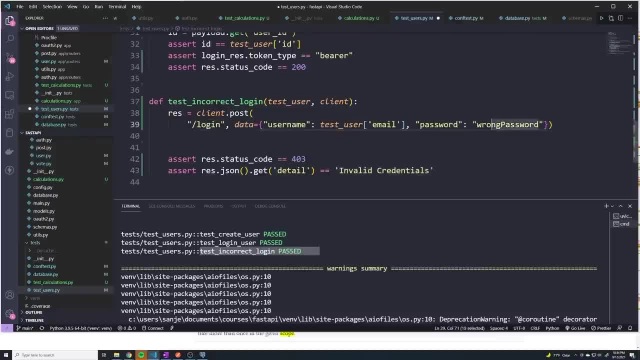 credentials. But not only do I want to test the wrong password, I also want to test wrong email as well, And I also want to test wrong email and wrong password and a few different things. So how do we do that? Well, we can use parameterize. 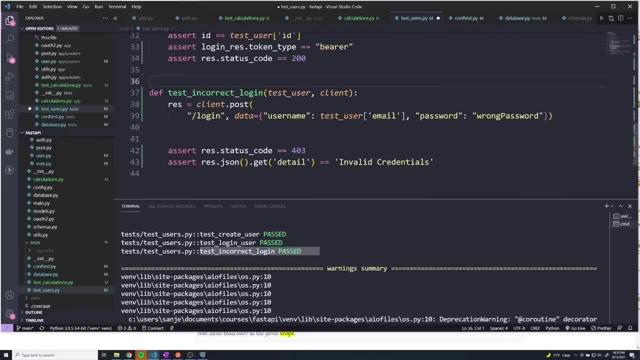 right. So let's import pytest, which we already have, And we'll define our decorator. So pytest, dot, mark, dot, parameterize. So what are the properties that we want to pass? we're going to give it the attempted email, the attempted password, And then we could also get the status code. 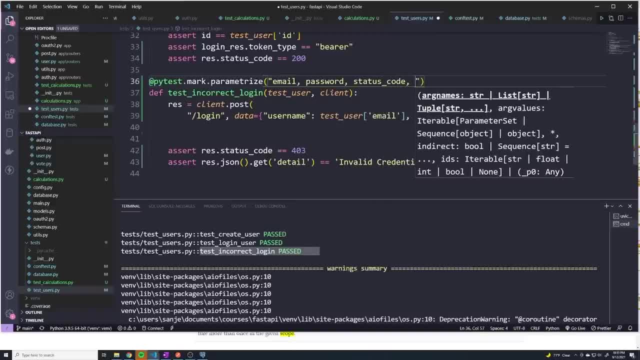 And we could also, you know, match on a specific detailed message. if you have a different detail message for wrong password, wrong email, but we don't, So I'm not going to include that, And then now we'll just give an array. 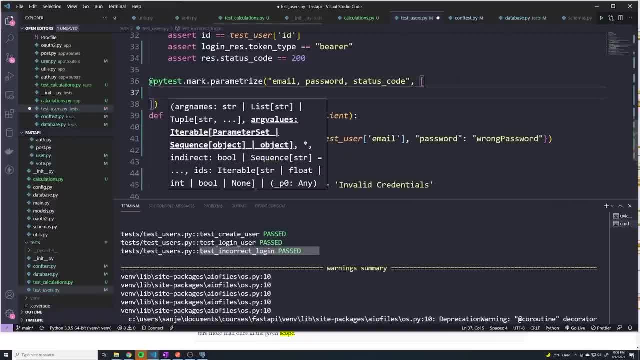 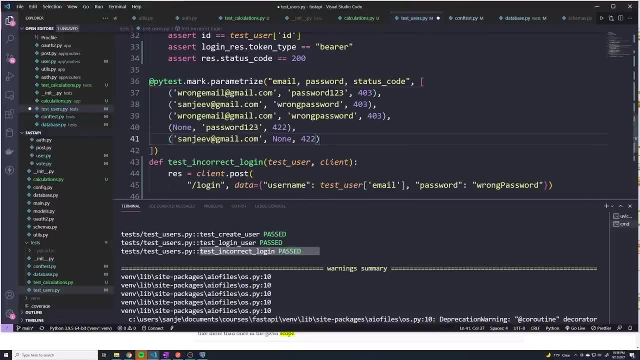 with all of our. Why does it do that? So, we'll hear, will define our tuples, And I'm going to copy and paste this part just because I don't want to have to make you guys sit through this. but I've got a couple of different test scenarios, So here I've got the email being: 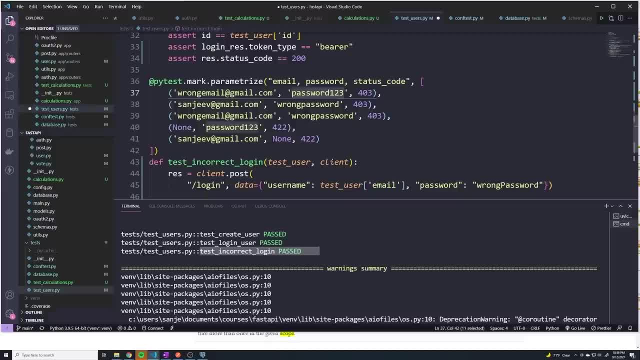 wrong email. at gmailcom. with the correct password, we expect a 403.. I've got the right email, wrong password. I've got the wrong email, wrong password. I've also got no password. sorry, no email. So if you put none, this is essentially leaving it blank. So, with this, set to none. 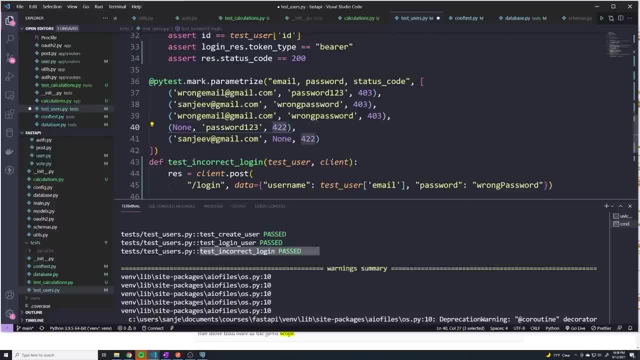 you'll see that our API actually will send a 422 because the schema validation fails because it expects a username or password, And then we'll try sending it with the correct email, but no password at all. we should get a 422.. In this case, because pydantic performed its validation. 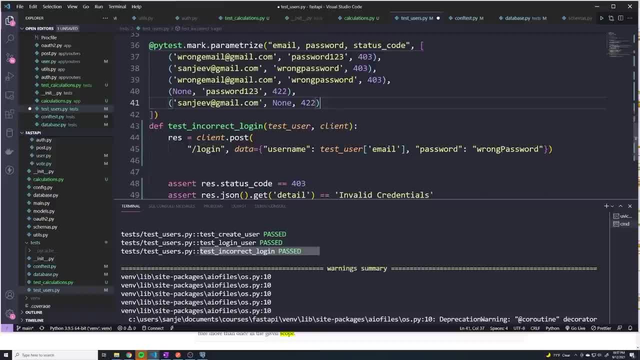 and found that it was missing fields. So that's what I'm doing here, And then we're just going to update all of this. So the email, we- Yeah, the email- is no longer going to be test user, It's going to be well, actually, we first of all, we have to pass it into our function. So email. 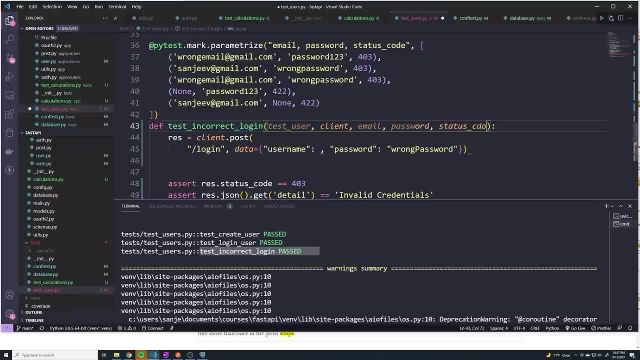 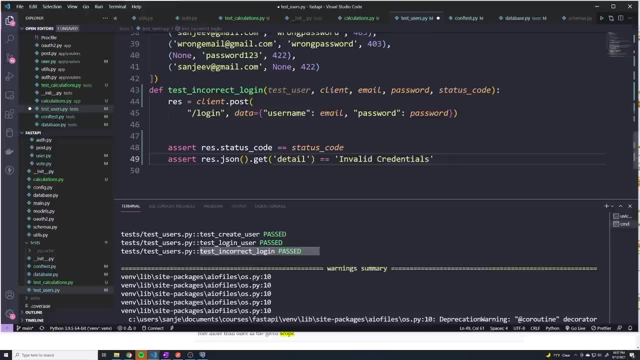 password and status Code. So we'll say email password is going to be password And status code is going to be status code And we'll get rid of this check Just because the invalid credentials won't apply when we get the 422.. Let's try this out now. 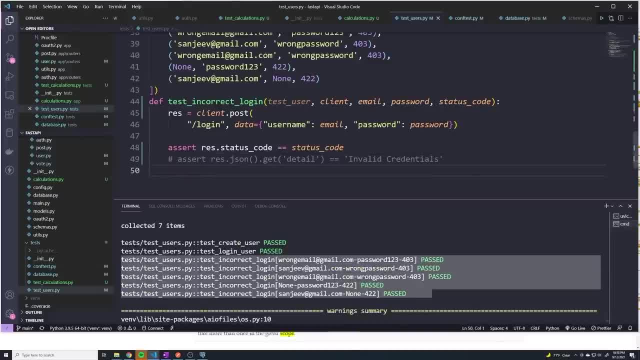 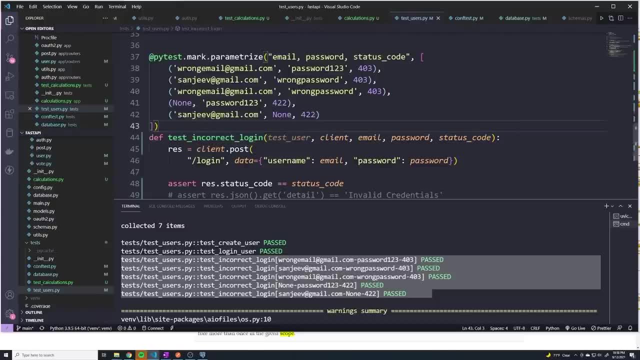 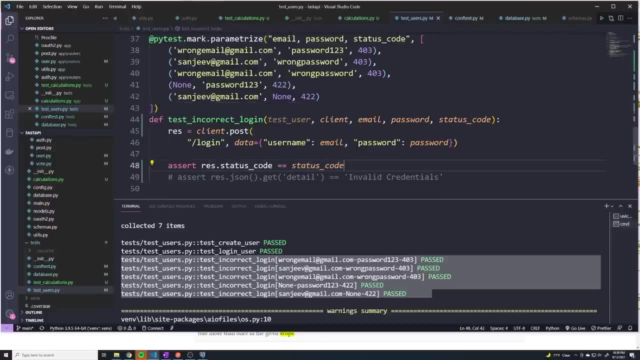 And we can see all of our tests have successfully passed. So we have now finally set up a test for making sure that, when a user does not provide the proper credentials, we get the right response code and the right data back And keep in mind guys, right In this case. I just set this up to be a very simple test, just. 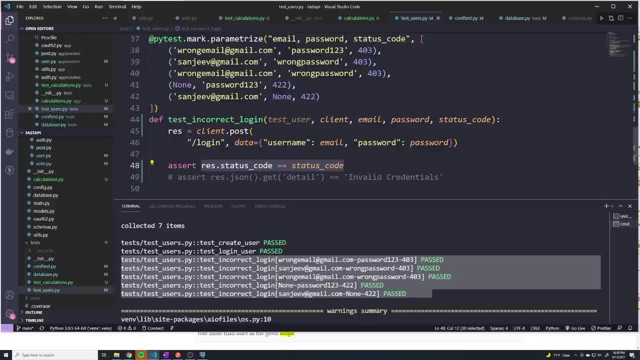 to check on the status code, But you could check any single field that you want. It's up to you. You can make your tests as specific as possible. You can make them a little bit more generic. It's up to you to decide on what you want to validate yourself. 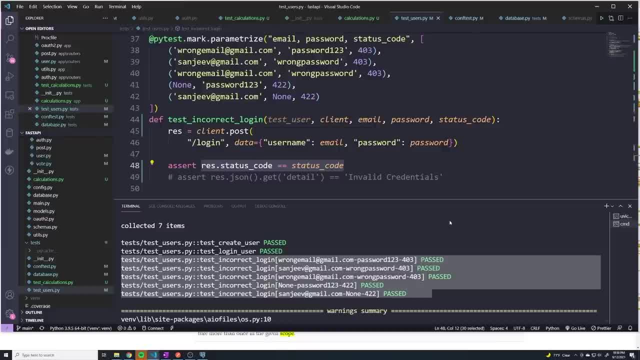 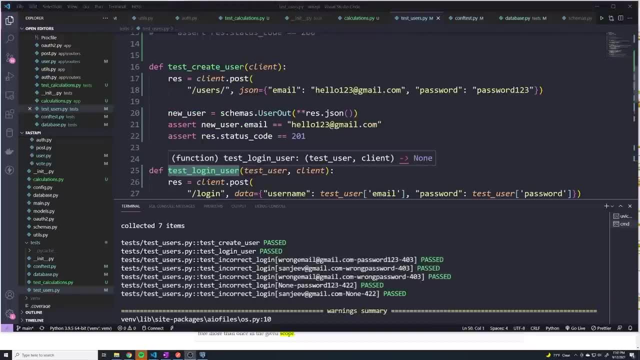 Like I said, I'm trying to keep this as basic as possible. Try to just make sure that we focus on how to actually create tests and less on the actual specific tests. That's all of the things that I want to do for all of the user tests. Let's move on to all of the post tests. So tests. 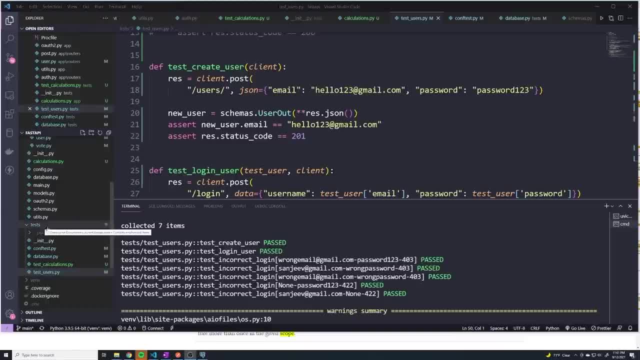 when it comes to creating, reading, updating and deleting posts, So I'm going to store this in a separate module, just to keep things nice and organized. However, you can keep everything in one file if you really wanted to, but no reason to do that, So I'll call this test underscore post. 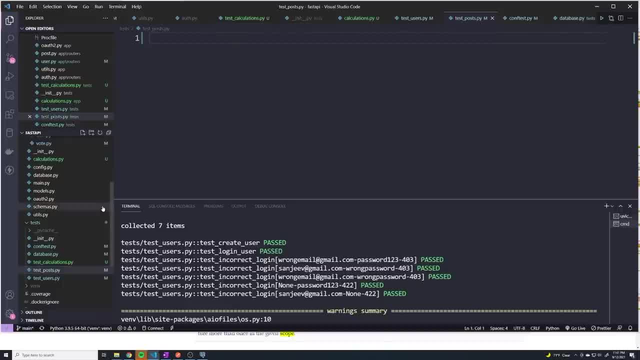 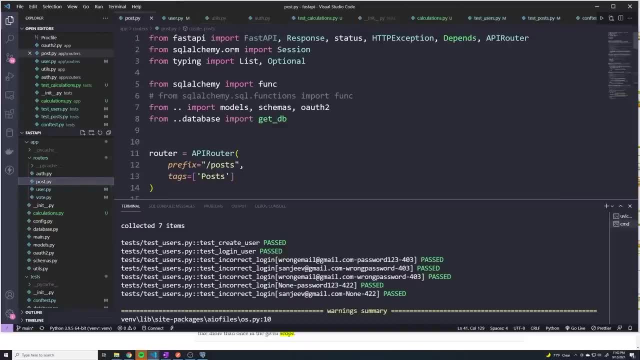 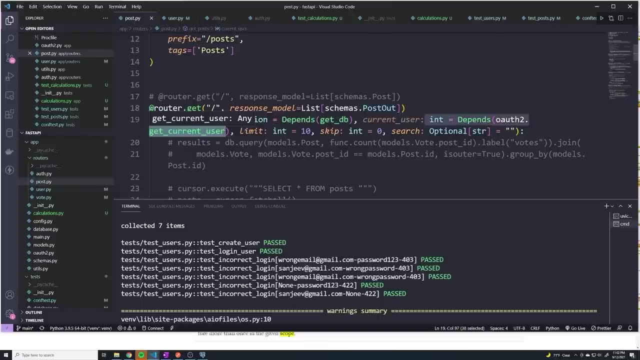 py. Now, when it comes to working with posts, we do have to deal with a little bit of an extra challenge, And that is, if you take a look at all of our post path operations, they all require authentication. So how exactly do we deal with authentication when it comes to testing? Well, 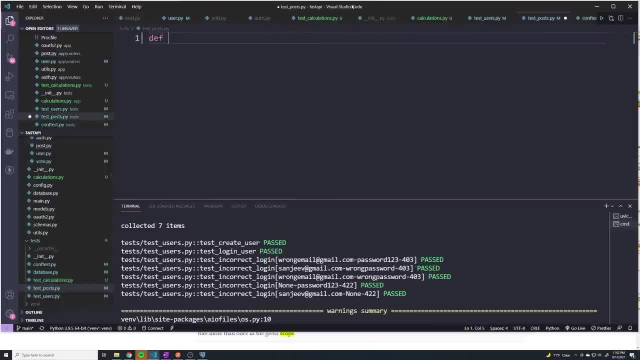 you're probably thinking: you know, we could, you know, define a post, define a test, and we can call this. you know, get all the posts that we want. So we're going to do that And then we're. 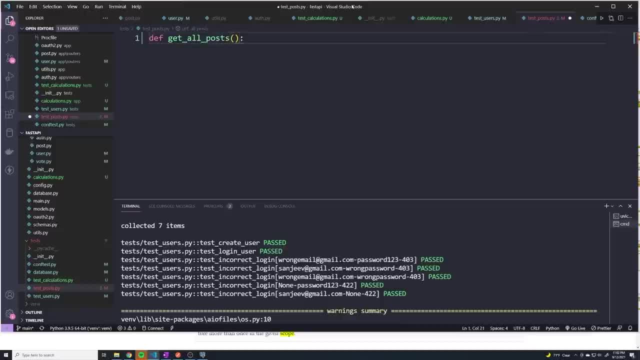 going to call all posts or something right, And then here we can pass in client And then maybe test user, We have access to that- And then we would just do: you know, client dot, post login, So we log in, we get a token And then, after we get the token, then we can. 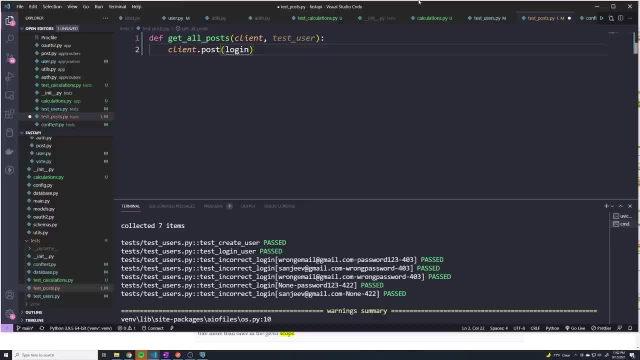 then we can make a request to post, And that is technically valid. But what I would like to do is I'd rather, I'd rather set up a fixture that automatically does this for us, But instead of- but instead of actually making a request to our API, I want to just import the. the method. 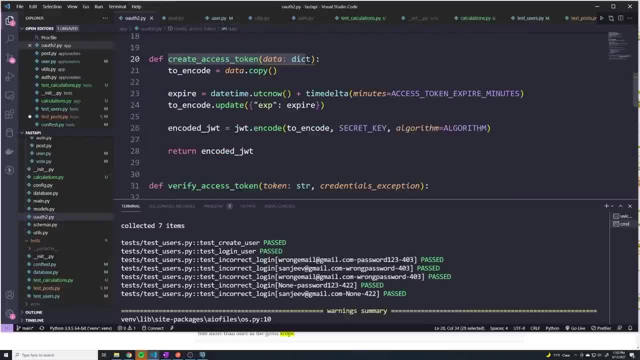 the OAuth two method for creating an access token, So we can just import this into our test so that we can actually fake our own token or create our own token without having to use the entire API and go all the way through back into this same exact method to get a token, because that seems. 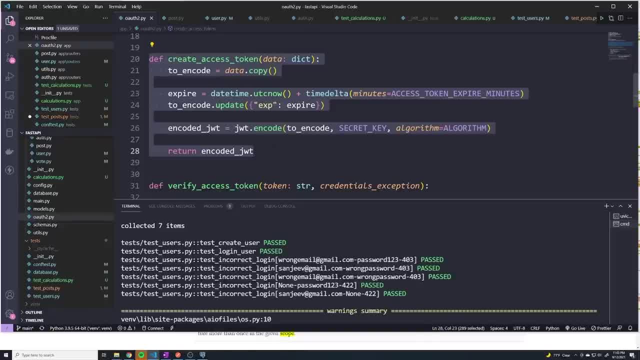 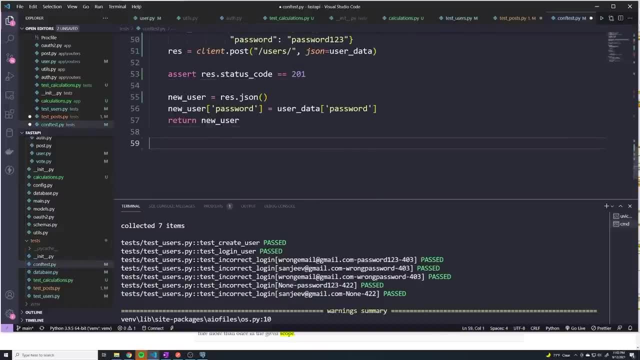 like a waste And we're testing a whole bunch of other things that we don't want to test in this specific test. So what we're going to do is we're going to go to comp test And I'm going to create a new fixture, I'm going to grab this And I'm going to call this token. 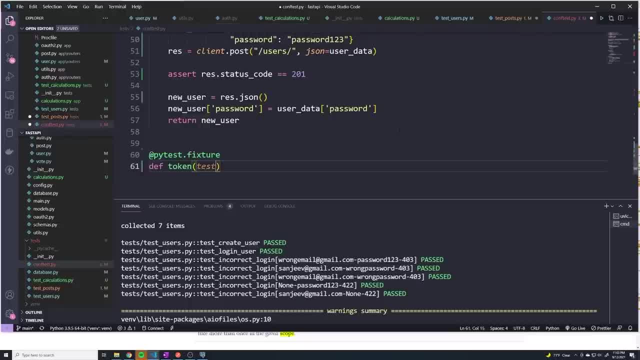 we'll say token, And this is going to be dependent on test user. So we need a user to get created first before we run this fixture, And what we're going to do is we're going to import this specific function right here. create access token from OAuth two. 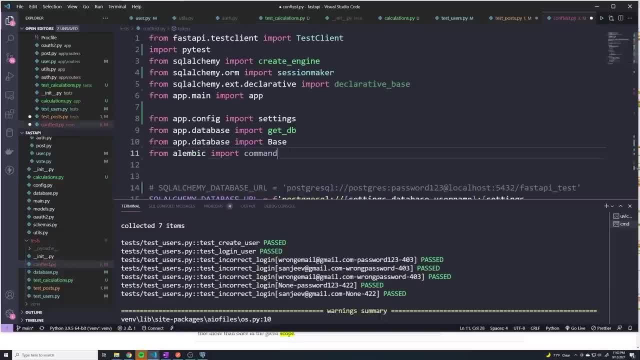 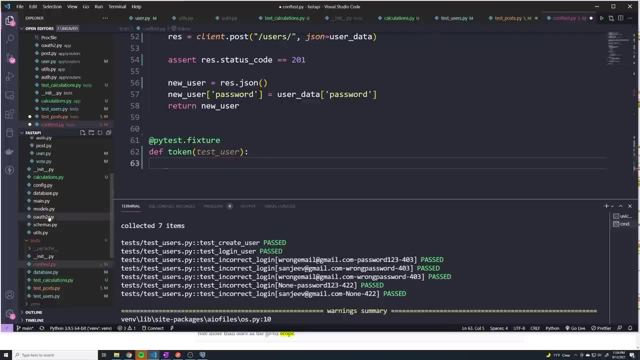 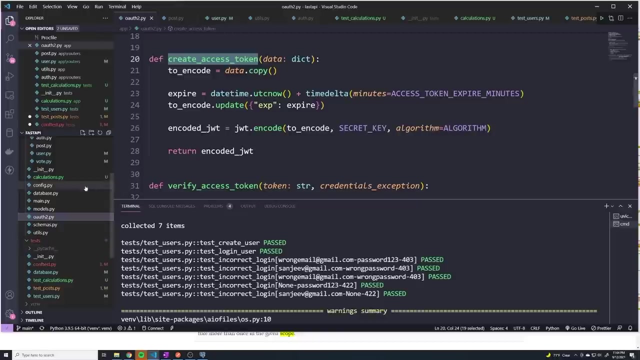 And so I'll go from app dot OAuth to import, create access token And just to quickly recap on how that function works. we pass in a dictionary, But I don't actually know what is in the dictionary, So let's go to. where is this? 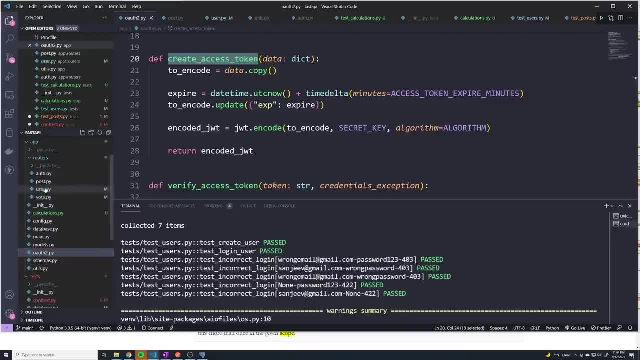 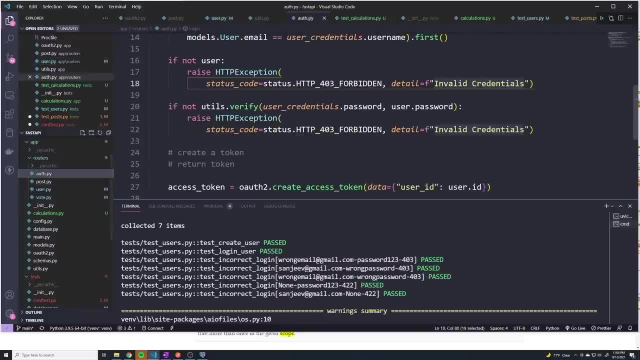 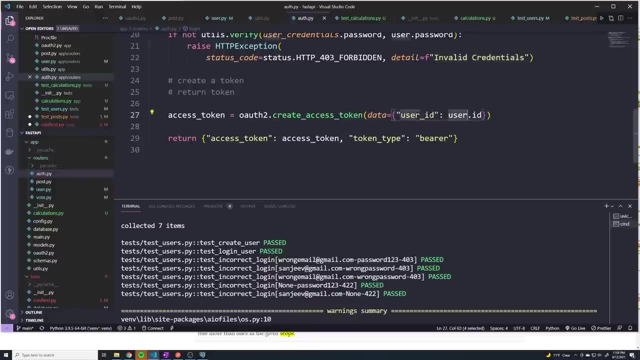 Who calls this? I think it's. no, it should be under users. Yeah, So create user. No, it should be under login, So under login, this is where we create the token, So we pass in data, which is just a property called user ID, and then we pass in the ID. 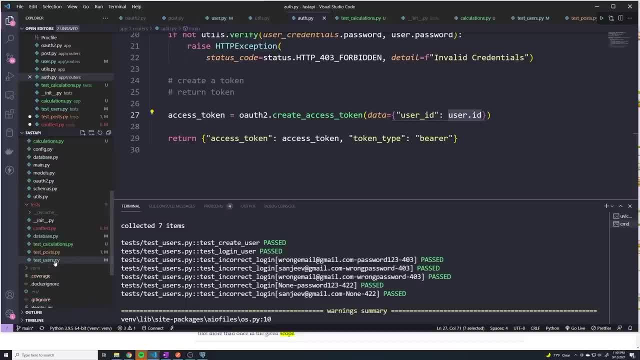 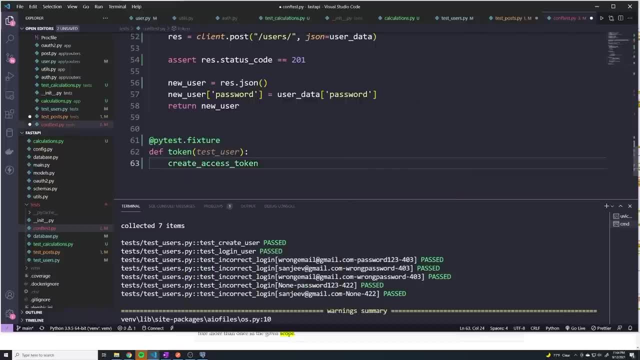 That's all pretty straightforward So we can do that. So I'll call create access token And it's gonna be a dictionary and we call this was a user underscore ID And we're going to pass in and we can get the ID of the user from test underscore user which is being passed in and we'll 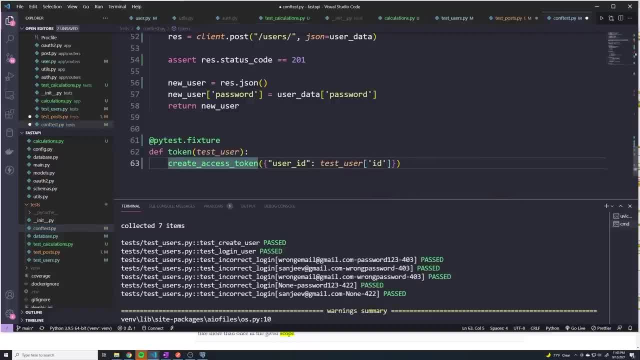 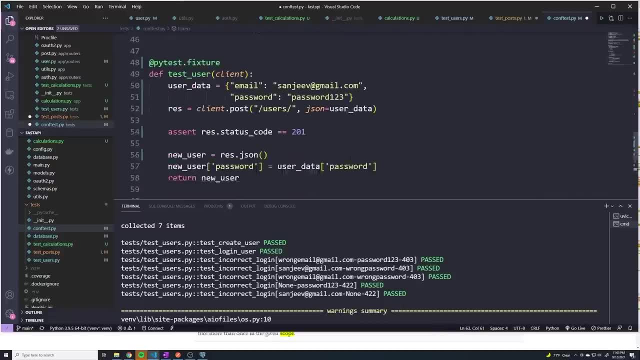 grab the ID property And we'll just return this. So this is going to return a token, And that's why we call this function token. Then what I'm going to do is I'm going to create a another fixture. I know there's a lot of fixtures here, But you'll understand why I want to do this. 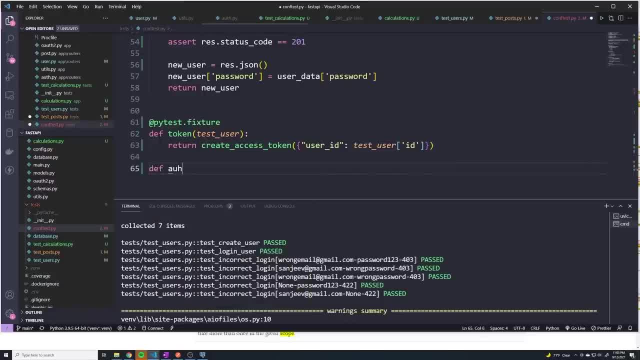 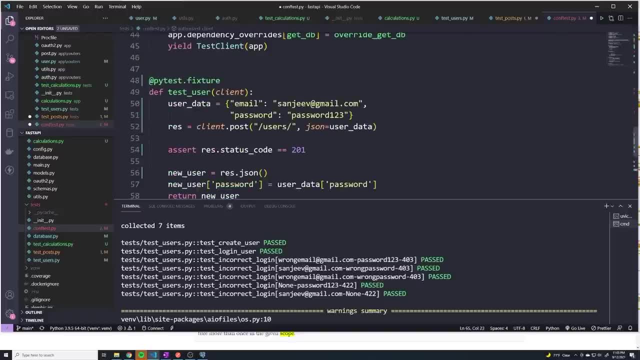 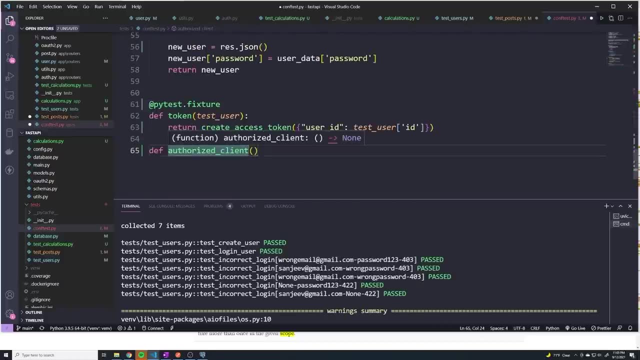 So I'll do def, Def, And here I'm going to call this authorized underscore client. The reason I'm calling that is if we take a look at our current client, this just gives us an unauthenticated client. this new fixture will give us a authenticated. 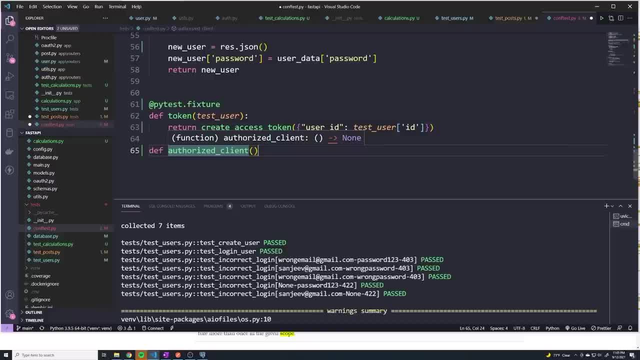 client. So anytime we want to deal with any path operations that require authentication, we can just call this client the authorized client instead of the regular client. So that's going to save us a lot of time And this is going to require the regular client. and this is going to require the regular client. 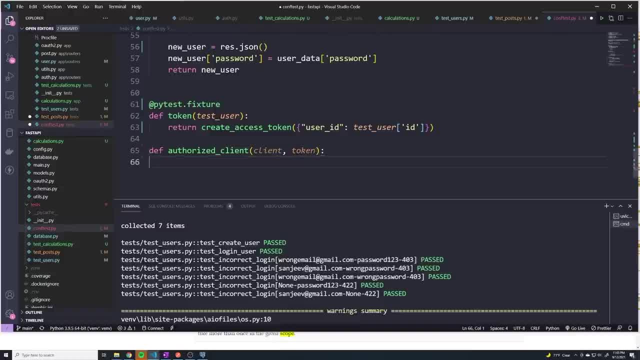 client and token because we need to get a token, Alright, so we have access to the original client- And what we can do is we can update the headers because we need to pass the token inside the headers. we do client dot headers And then we have to pass in a dictionary And what we want. 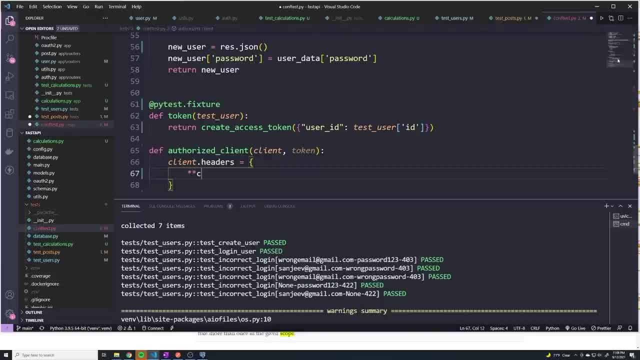 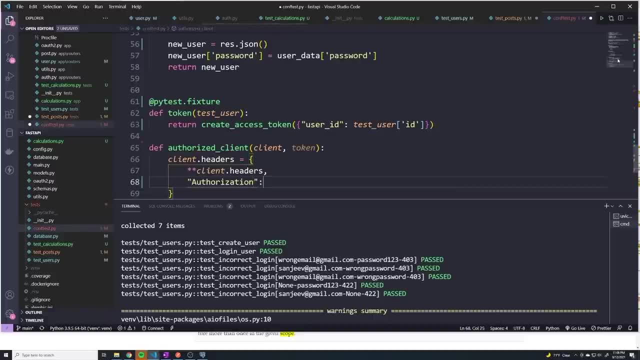 to do is we want to spread out all of the current headers, So we do client dot headers, And then we want to add one more which is going to be the authorization, And this is going to be an F string, because we need to add the word bearer before, and then we can pass in token And then 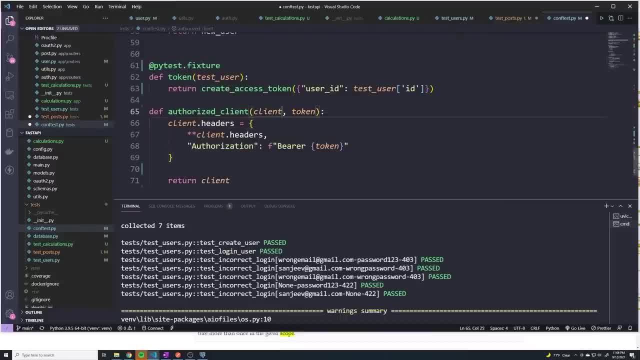 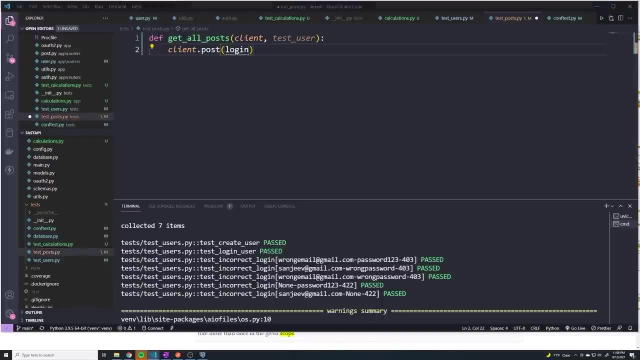 we'll return this client. So it's basically taking the original client and then just adding this specific header that we get from the token fixture. That's all. And so now, when we go into get all posts- and I forgot to put the word test before it- Instead of client, we want to import authorized. 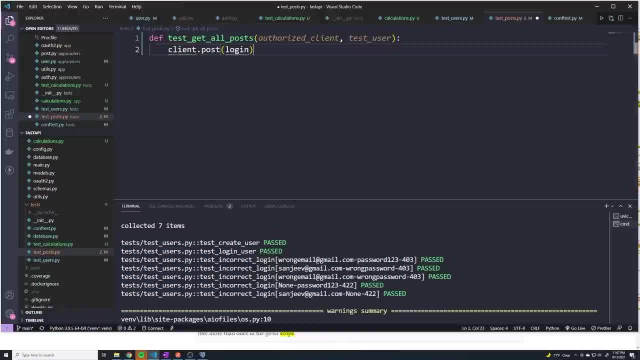 client. We don't necessarily need test user At this point. it'll automatically get called because you know, this calls token, token calls test user. we only need to pass in a test user if we want access to specific user data, but we're not using any of the information. 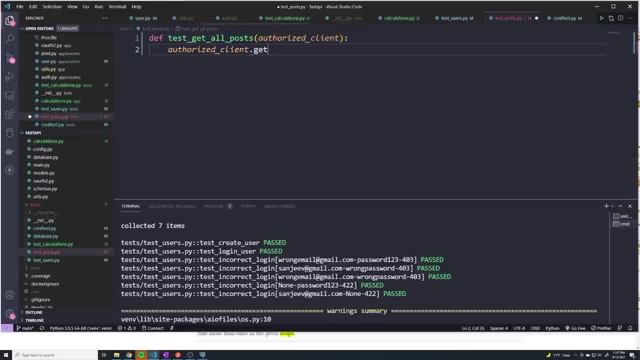 at the moment. So I'll do. authorized client dot get is going to be slash posts. We'll set the response equal to that And we'll just do a print res dot JSON just to see what that looks like. And I believe the status code should be a 200 because we're retrieving data. So I'll do a. 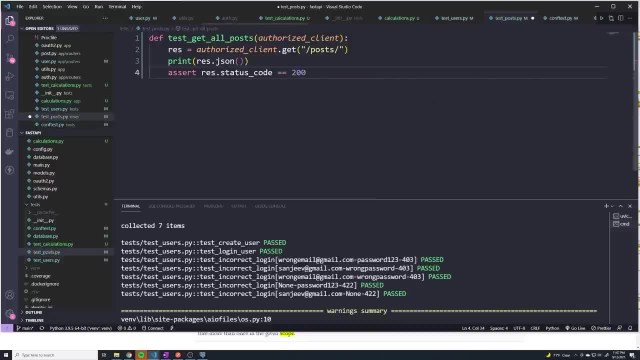 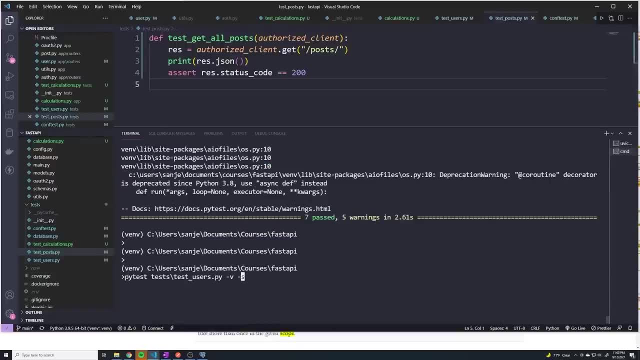 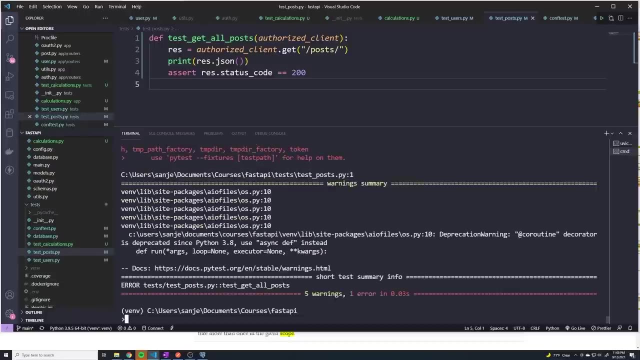 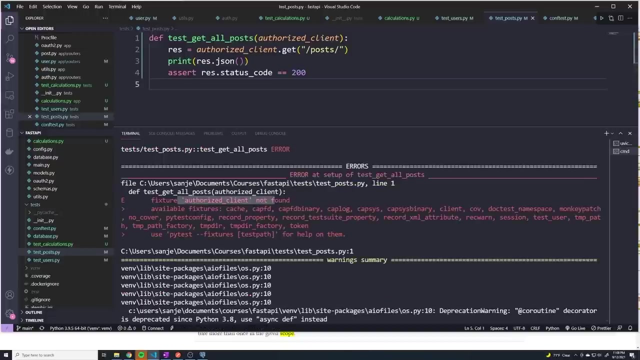 res dot status code equals equals 200.. Let's just take a look and see what exactly is happening here And now. it's going to be test posts And we get an error. So let's see what happened. Authorized Client not found. So let's- I think I forgot to save. Let's try this again. 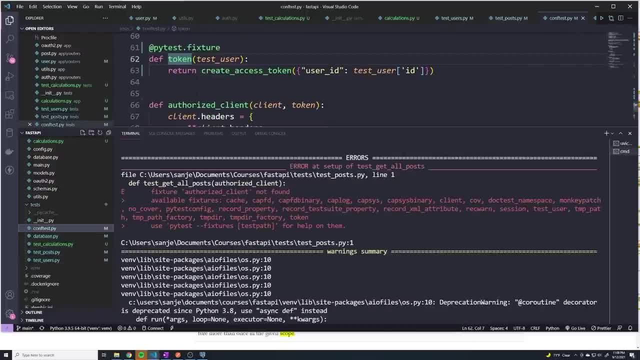 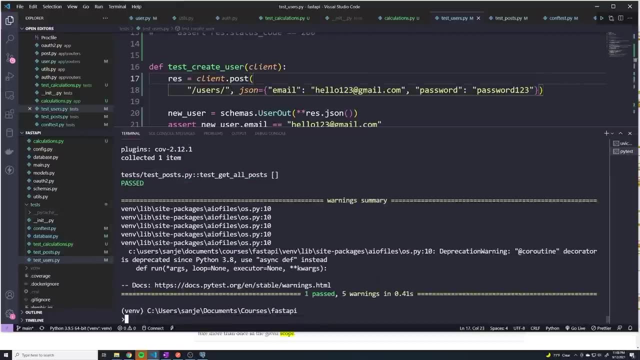 again And I forgot to turn this into a fixture, So right now it's just a regular function. So let's make sure I add the fixture there So it's accessible to everyone. And now, if I run this- okay, so one passed- let's take a look at the data that we got back. So when 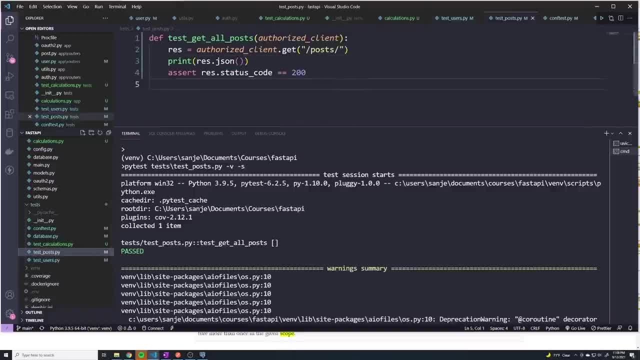 I did a print print of res dot JSON to see the data. I got an empty array. And the reason we got an empty array is that there's no test data in our database. there's no test posts, Gino, so we're going to have to actually create some test posts before we run this. 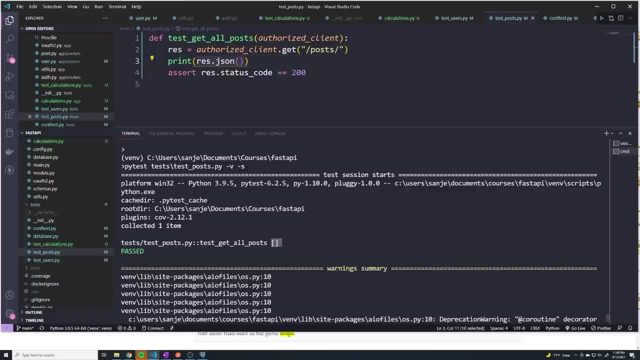 test that we can actually verify that we got what we expected to get. So, just like we did with the login user, where we created a test user before, we're going to have to do this with our posts. we need to create a whole bunch of posts and then verify that we are. 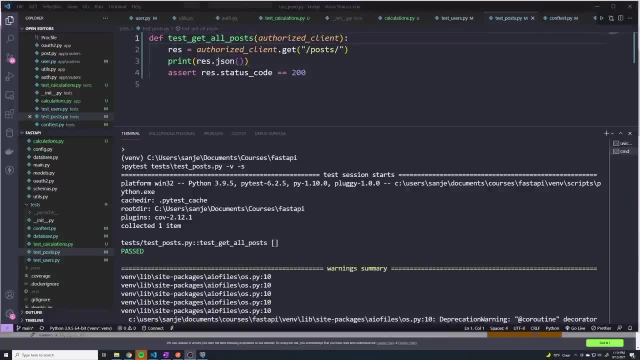 able to retrieve those posts. So we'll tackle that in the next video. So let's create a fixture that will create a few initial posts so that we can actually test retrieving all posts, And we can use that same fixture for performing a few other tests, So things like updating a post, right? 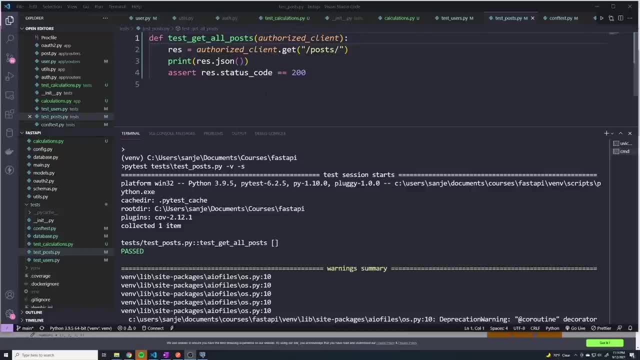 we would need to have a post in our database to update a post. same thing with deleting, same thing with getting an individual post. So this fixture is definitely going to be very reusable across a lot of our tests. So let's figure out where we want to store our 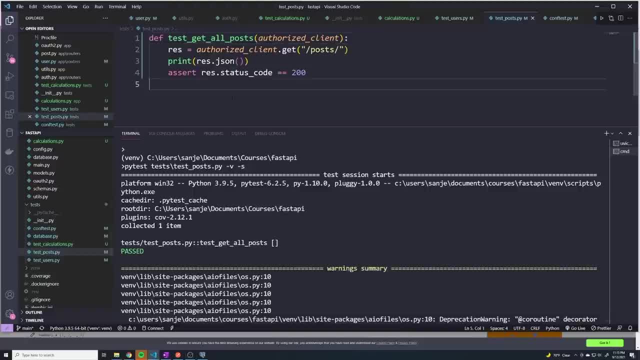 fixture. we could keep it in our test app posts: test underscore post file, because all of our posts, all of our test posts, sorry, our tests, our fielded tests for post data. I guess if you want to call, that will require. 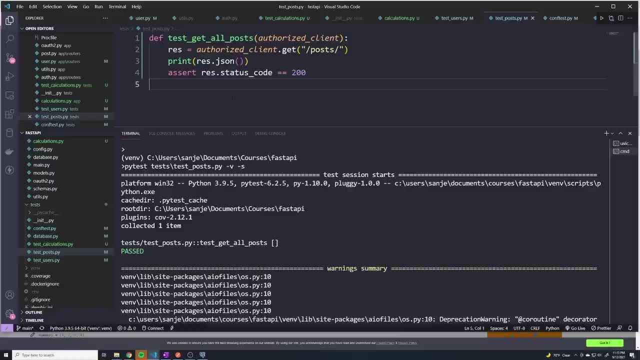 that fixture probably. However, there are going to be other tests in our application that will need posts initially. So when you want to vote, we need a post already in our database. So I'm actually going to put it in our comp test file so that you know everyone. 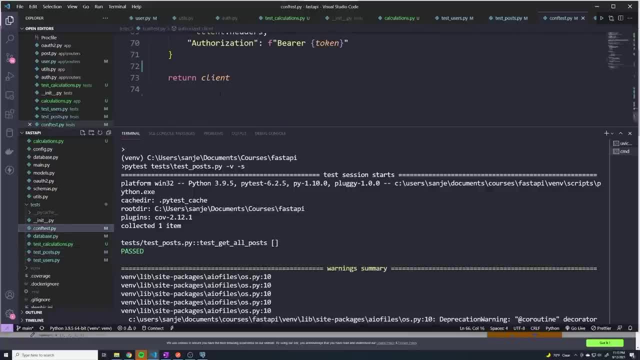 has access to it. Well, technically, anyone can access any fixture if they import it. but having it in the contest file makes it simple, because we don't have to import it. I'm going to put it in here And I'm going to this. this fixture is going to be a little. 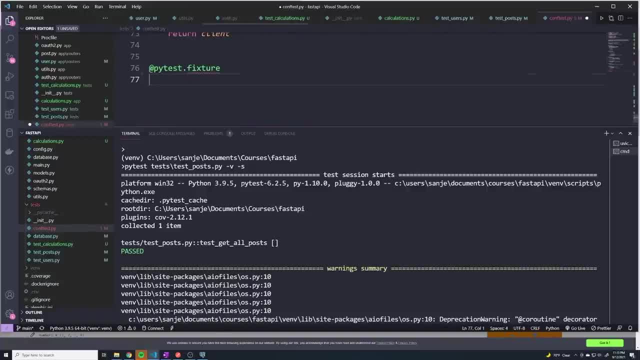 bit different, just because we're actually going to create the posts in the database ourselves. So here I'm going to call this test underscore posts, And so what we need is a couple things. So first of all, we need a test user, because if we don't have a user, 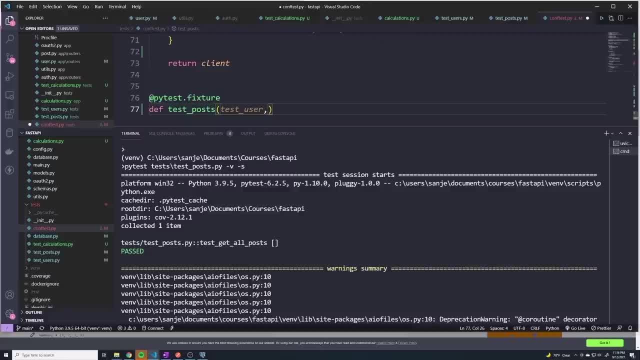 we can't create posts because all posts need to be associated with the user. Since we're going to work with the database, we're going to pass in session also, All right, and let's define some post data. So I'm going to create an array of dictionaries And I'm actually 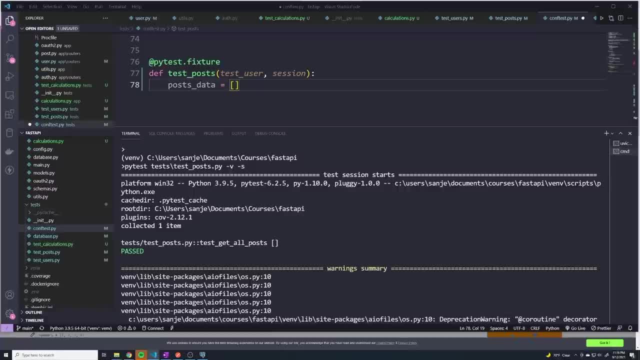 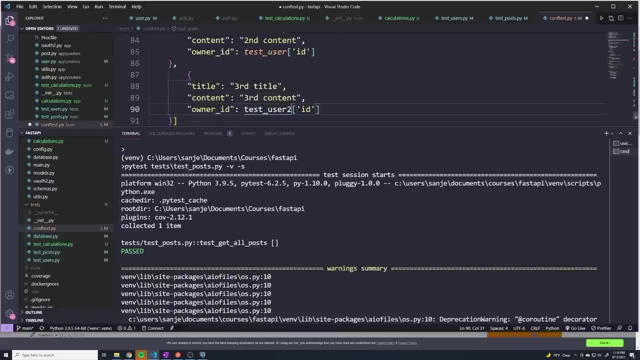 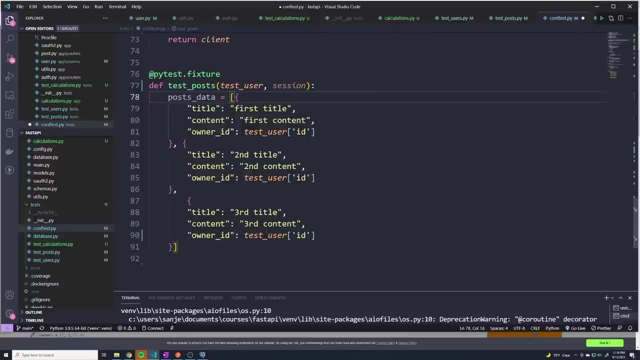 going to copy and paste some data, just because I don't want you guys to sit and watch as usual. All right, so what we're doing here now is we're creating three posts. So in this post data I have an array, or sorry, a list, and then a dictionary, And then here we're providing. 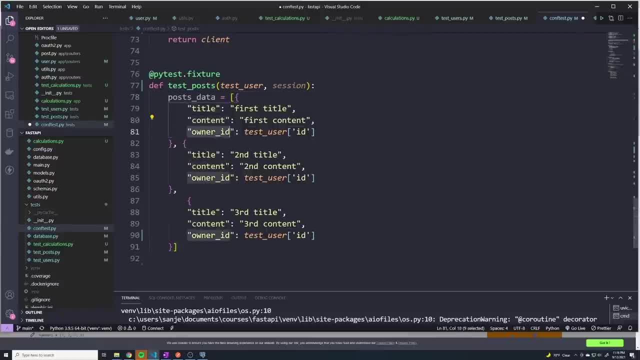 the title and the content and the owner ID. Alright, so that's going to create a post And we're going to the owner ID from the test user fixture And we're just gonna grab the ID from that. So we're saying the owner ID and then I'm just going to create another. 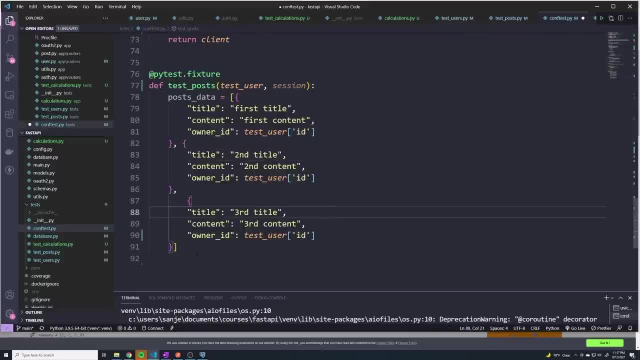 post here and another post here, So the same user is essentially creating three posts, And so now, since we have access to session, we can actually just directly tap into our database and create that information for us or those posts. So we can do well the when. 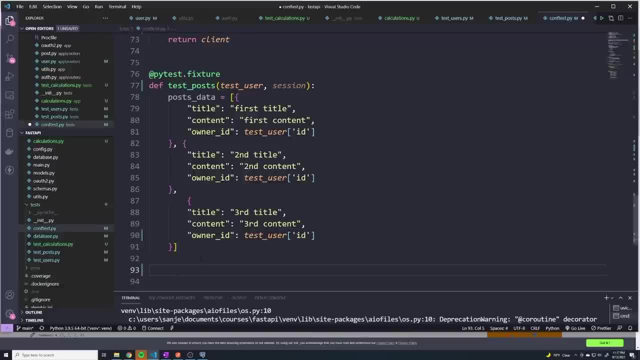 it comes to SQL alchemy, If you want to add multiple entries into a database, we have access to the add all method, So we can call session dot, add underscore all, And then here we have to pass in a list of user models. So we would. this would be, you know, schemas, not schemas. we'd actually 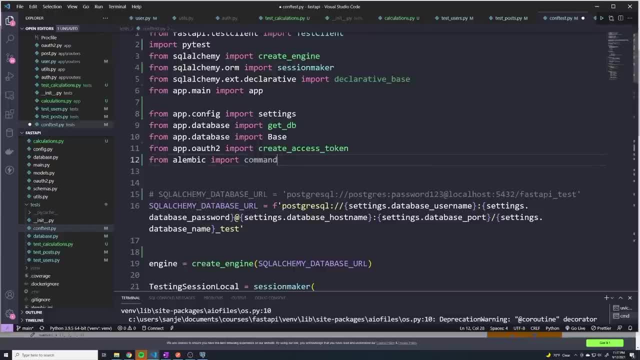 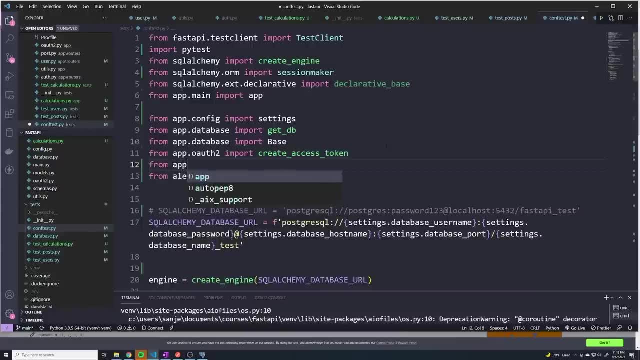 have to import models, So I'm going to import. Do I have models already in here? doesn't look like it, So I'll import that as well. So we'll say from app dot. we'll just say, from app, import models. And I can say: 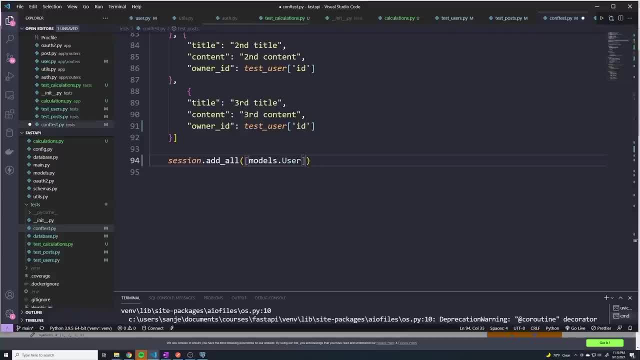 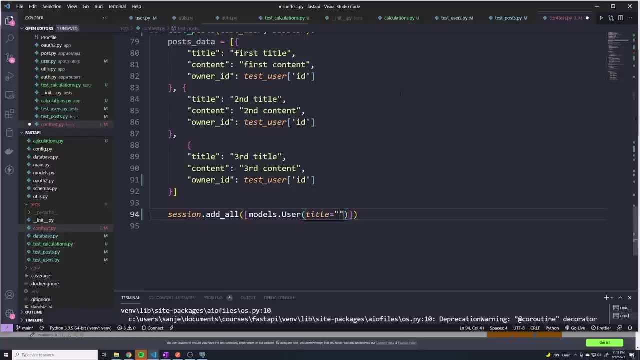 models, dot. user. So we'll create a new user model And then we have to pass in all of this data. So right, we would need to be: title equals, you know, blah, and then then content equals blah, And then we'd have to do another one. So I'd copy this, paste this in here. 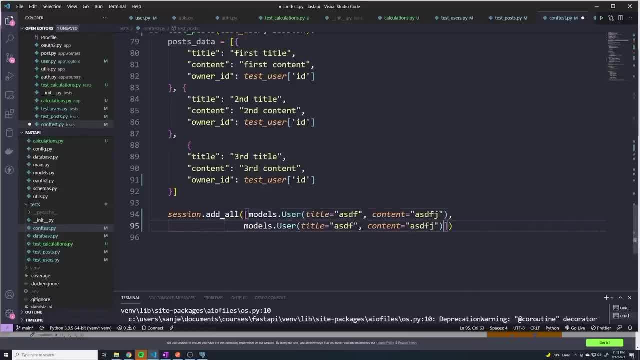 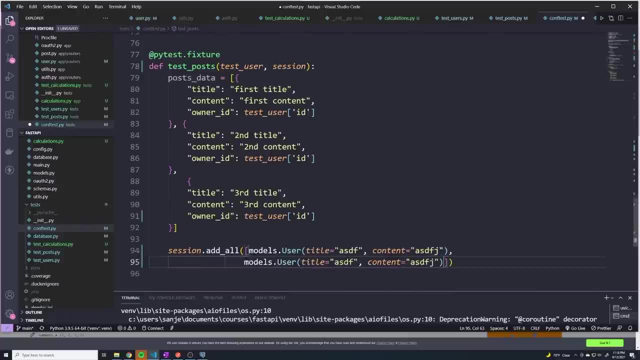 And so on, And then this would add it all at once. Now I can manually hard code this, This value into here, just to kind of keep things simple, And I could do that, And actually I will show you how to do that, just just to in case. but I'll show you what I did when. 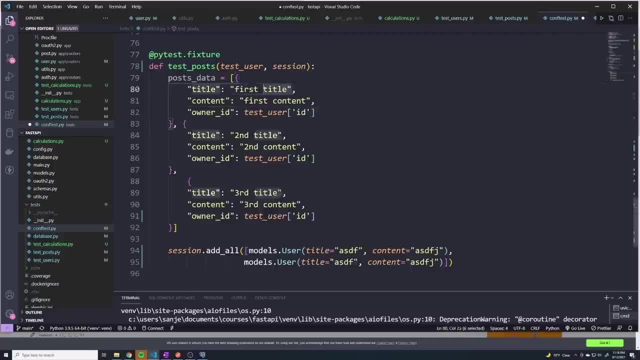 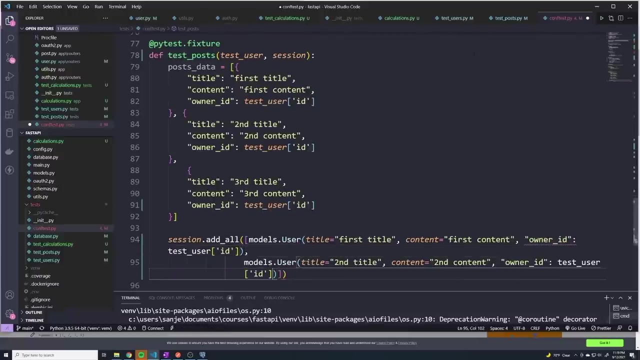 I was doing a dry run So I'll copy: the title is going to be set to first title, The second title is going to be here Content and second content, And then the owner ID is going to be the same for both, luckily, while all three actually. 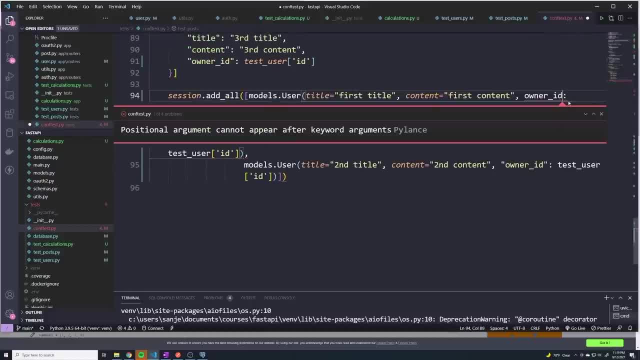 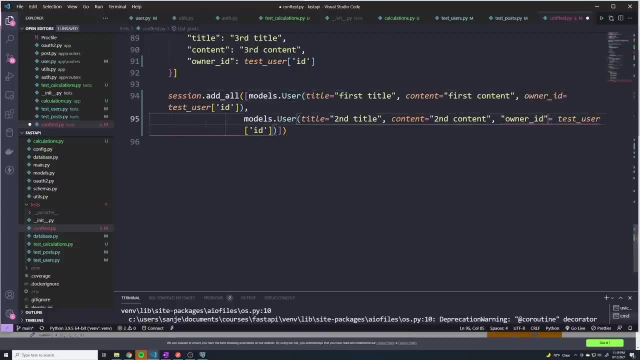 And that's not in the right format. Oh, don't do that. It should be equals And the same thing here, And if we wanted to, we can copy this last one and then put the third one in. This will be called third title, Third content. Alright, let's save this. The auto formatter did not. 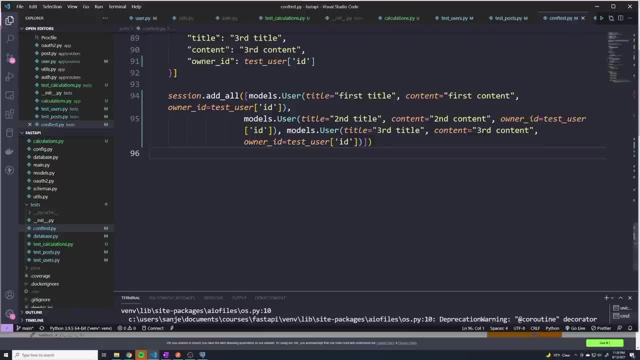 do much to help me out here. It still looks pretty ugly, but that's okay, And so that's one way of doing this. So it'll add it all and then all we have to do is just do a sessioncommit And then to get all the data back, I can just do a read all and then all, and then we can. 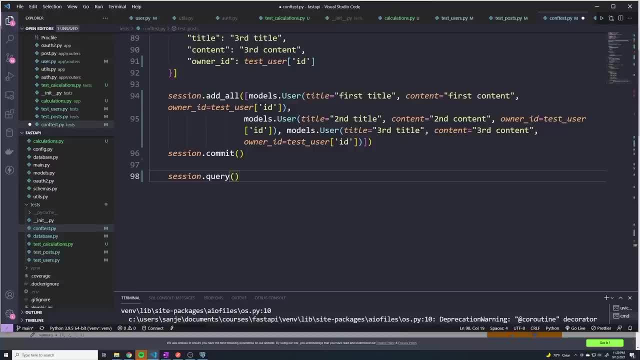 do another one, Yeah, Okay, so let's just do that, And it should be equal. And then the a session dot query And we'll just say models dot post. Oh, this should be user, by the way, not, I mean, this should be post, not user, because we're creating a post and not a user. 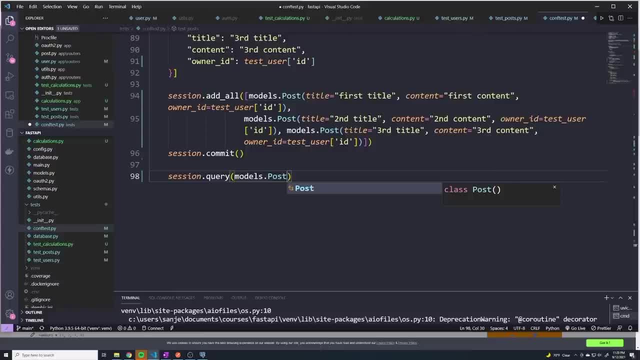 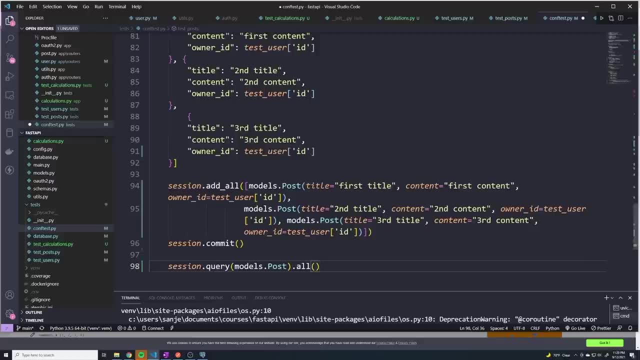 was a models dot post And we can just grab all of them Now. if you wanted to be able to take this dictionary and convert it easily to this format. there's a couple of things you have to do, But technically you could just leave like this and it'll work fine. But just to this is a little. 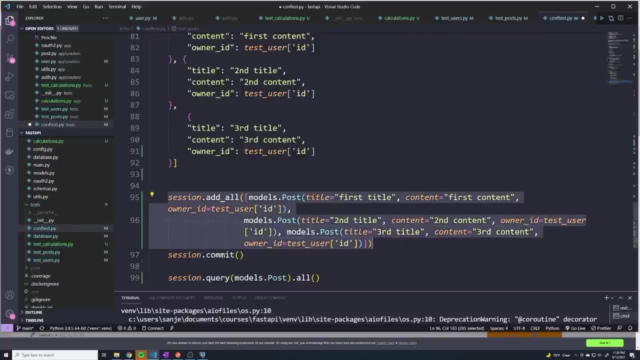 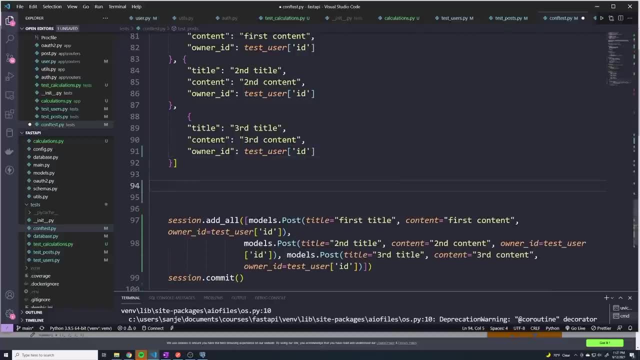 bit more of Python than anything else, If you didn't want to hard code it in like this- because at this point we don't even need this dictionary- But if you wanted to take this dictionary and convert it into a list of user models or, sorry, post models. what we can do is we can use the map. 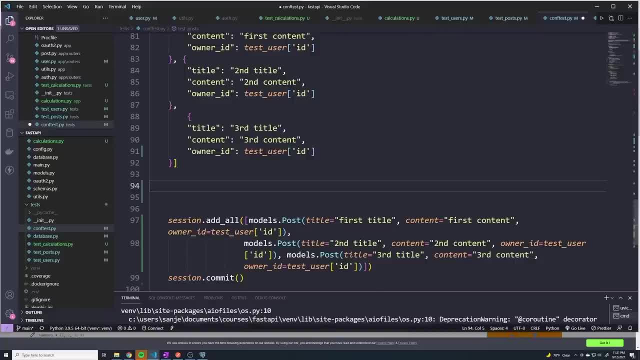 function, And so the map function works like this: You call map, then you call some function that you define yourself, And then you call the posts underscore data list that we have up here, And so this function, what it's going to do is it's 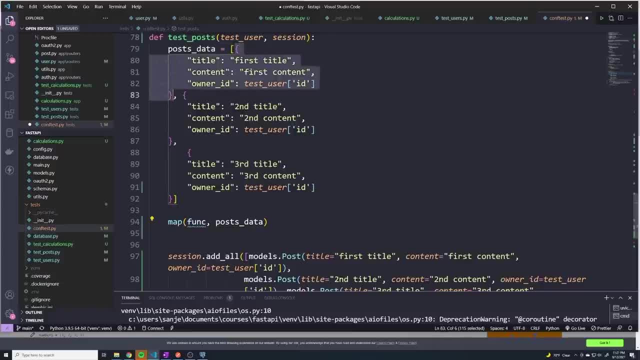 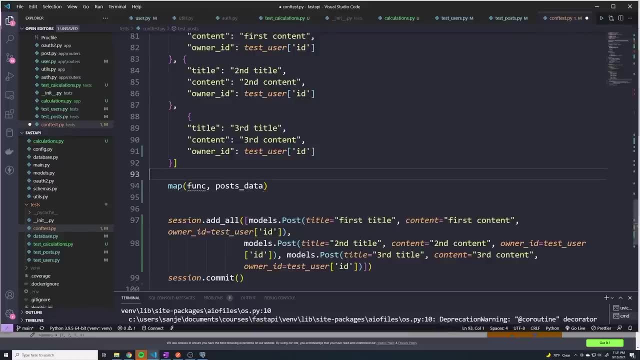 going to iterate through this list And it's going to take each item in the list, which is a dictionary, and it's going to convert it into a models dot post. So how exactly does that look? Well, let's, first of all, let's rename this And I'm just gonna call this: maybe create user model. 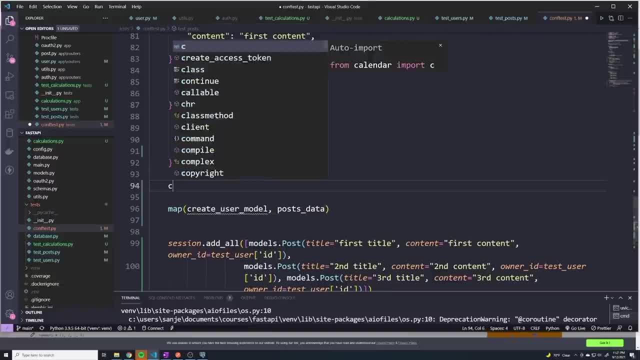 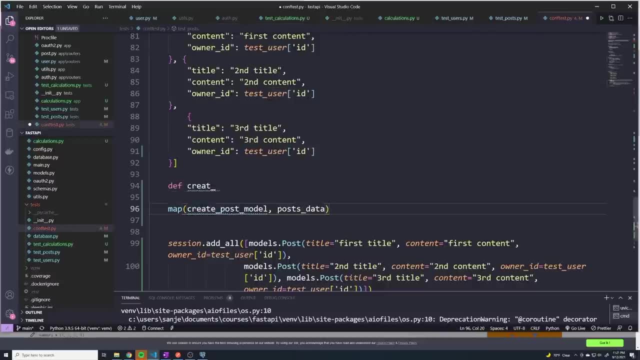 And I'll define a function up here And I don't know why I keep saying user, it's a post reading posts, not users create post underscore model And this is going to get passed in some some some object, but technically what's going to? 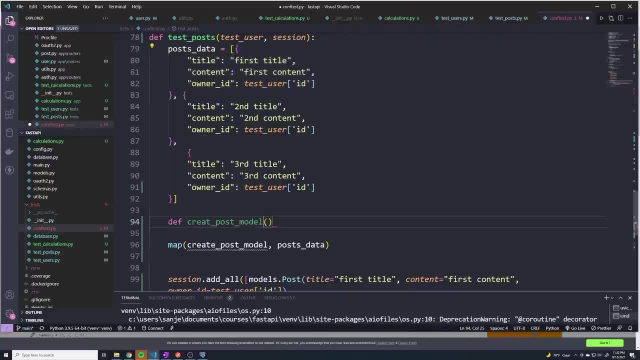 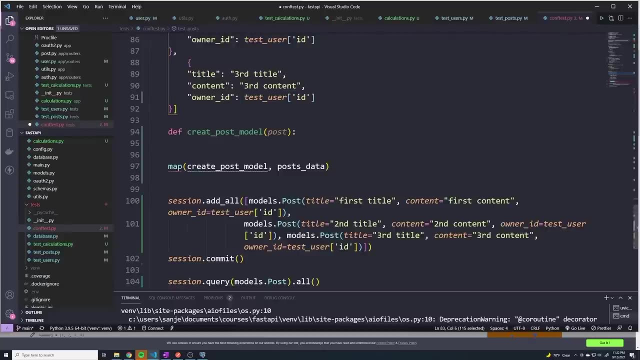 get passed into this function is each dictionary, So I'll call this post underscore data. Well, actually don't call post data, I'll just call this post. And so we have to put the logic of converting a dictionary into a post model, And that's pretty easy. All we have to do is just say: 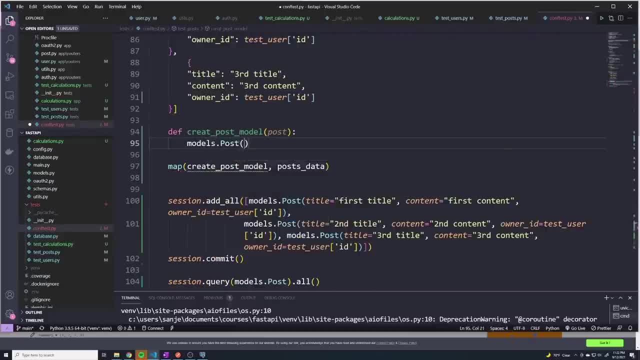 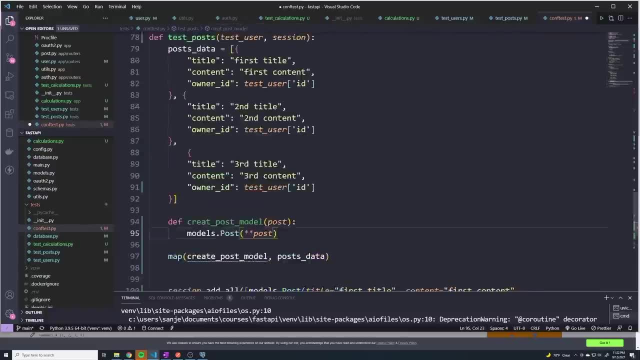 models, dot, post, And then we take post and then we spread it. That's it Right. So what's happening here is we're taking the dictionary, which is what it's going to get passed into here, And then we're taking it and spreading it, So it looks like it's going to get passed into here. 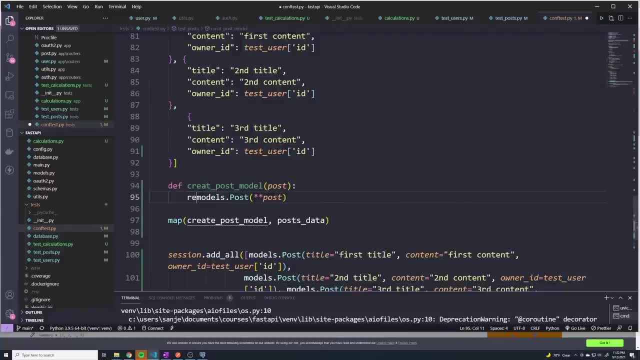 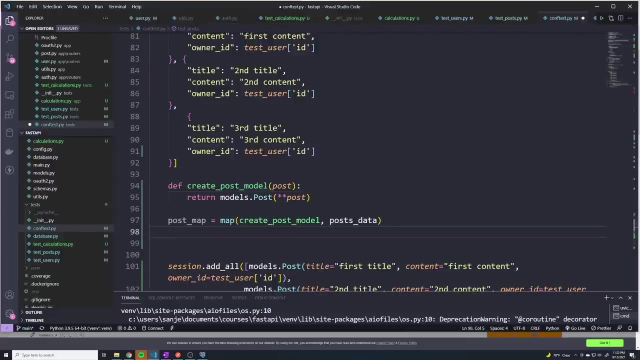 So it looks like title equals blah, content equals blah, And then we can just return that. And then this map, we just set it equal to some variable. I'll call this maybe post map, And I'm forgetting an E. Okay, so then, so that's going to return, So that's going to 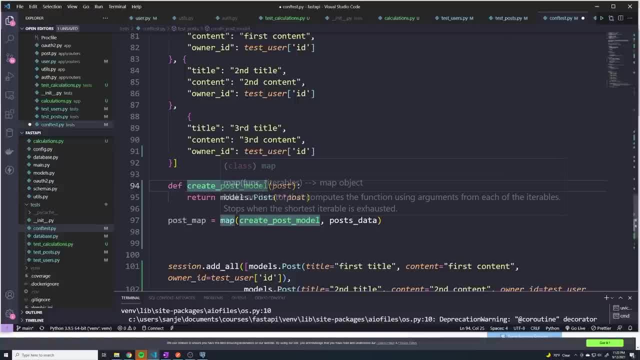 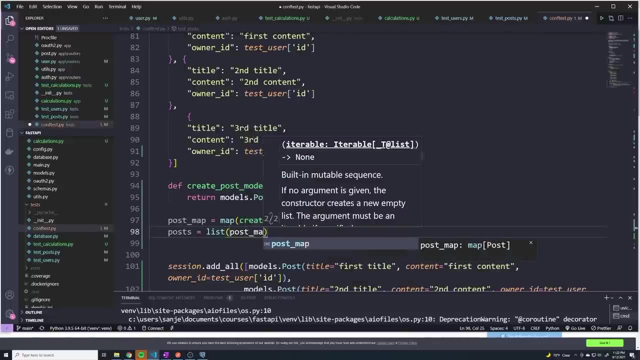 so that's going to essentially convert all of those two user models, but it doesn't return a list. it returns a map, which isn't quite the same thing. So to convert it to a list, all we have to do is then say posts equals. we just say list and then post underscore map. So that'll convert. 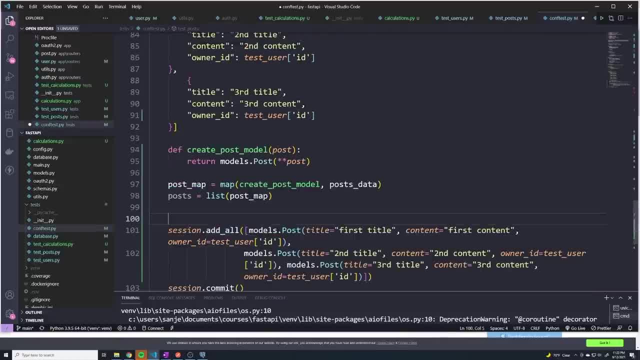 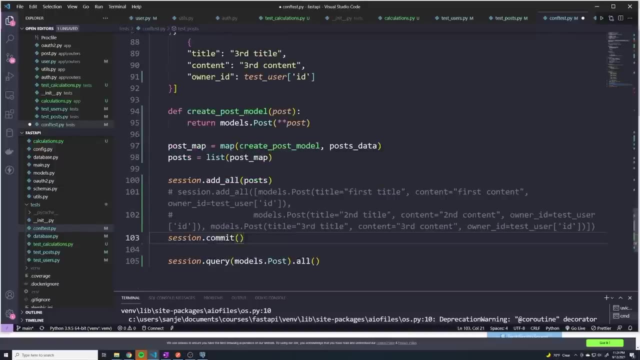 it to a list And then under a session dot, add all. instead of hardcoding those values, I can just say session dot: add underscore all And I just pass in posts And we can just comment out this line right here. Either one works, choose whichever one you like. I don't really care, But this is all. 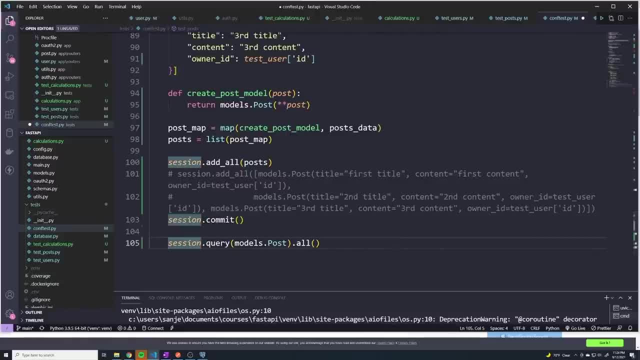 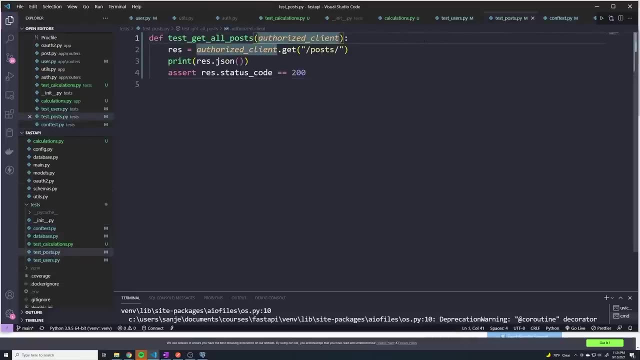 we need to do? we just have to return this. I'll save this as posts And we'll return posts, And that should create three posts in our database. And so now, if I go to test posts and make this reliant on what did I call it get test posts. 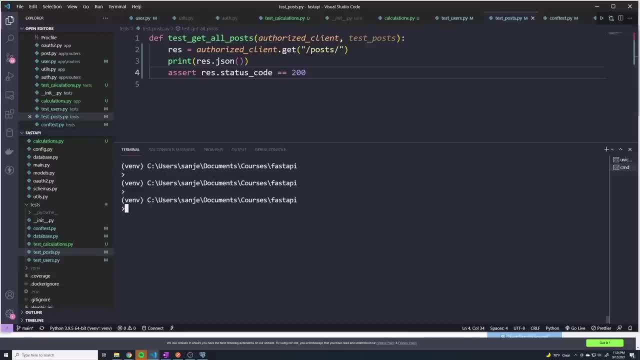 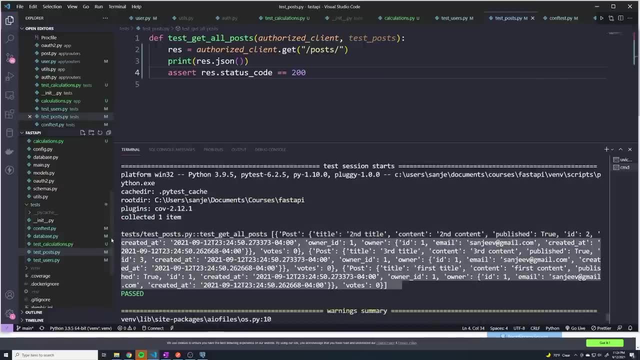 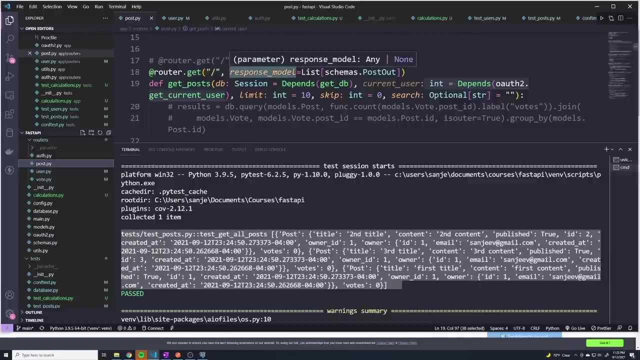 If I then run this, you can see that we did in fact get multiple test posts And it's up to you to decide what checks you want to perform. If we go to our post route and we take a look at the schemas, you can see that it's going to be of type list of schemas that post out a list comes from. 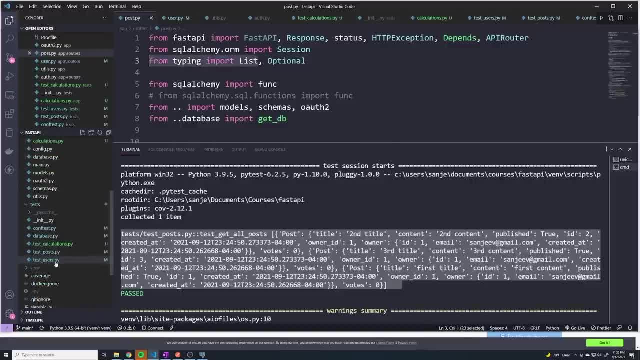 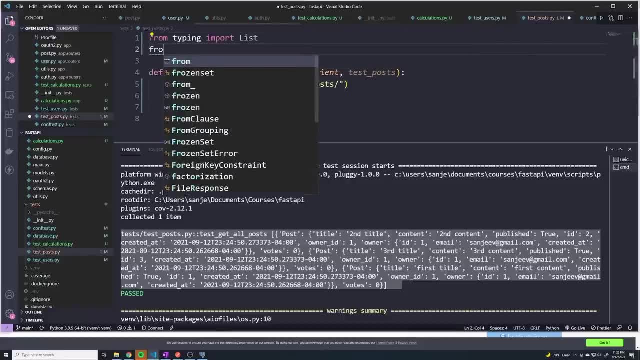 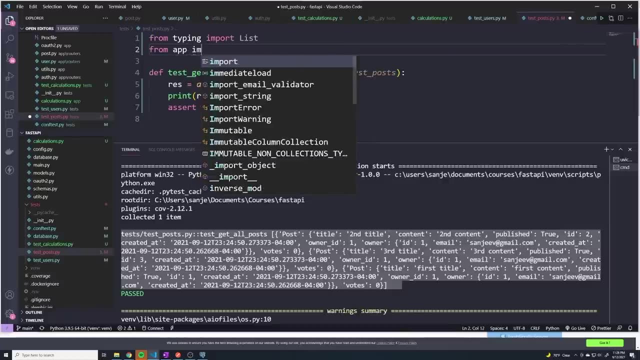 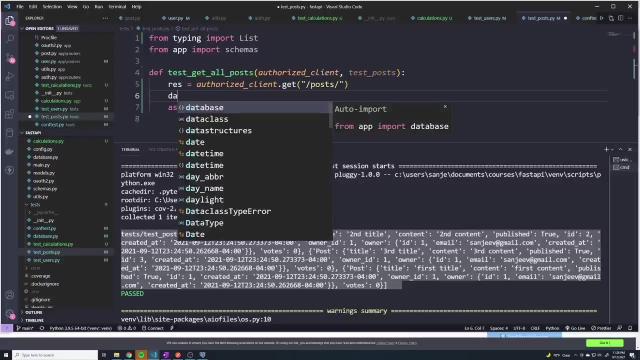 the typing library. So let's see if we can actually do this. I never actually tried this with this, But I think it should work, So I will import that And then we'll also import from app from app: import schemas And. 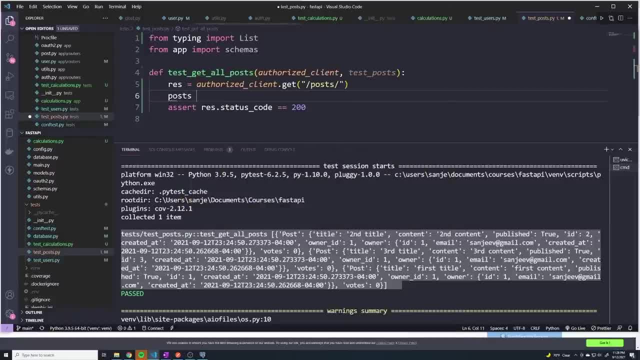 I'll just say posts equals res, dot JSON. And I'll say actually, schemas, dot. what is it post out? Yep, it's gonna be post out. I don't think that'll work, Because, Yeah, I don't think that'll work Because we're this is expecting one. 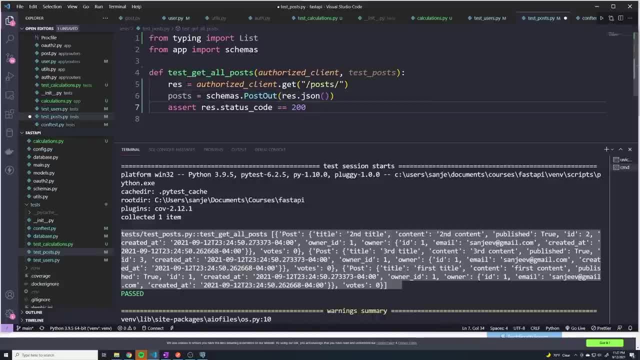 individual post, but this is going to be a list of posts, So I don't actually I wonder if I can do: Yeah, we'd have to do this manually, like we'd have to iterate through it, And then I basically copy it out, And I think that would just take too much work, So we'll leave this section. 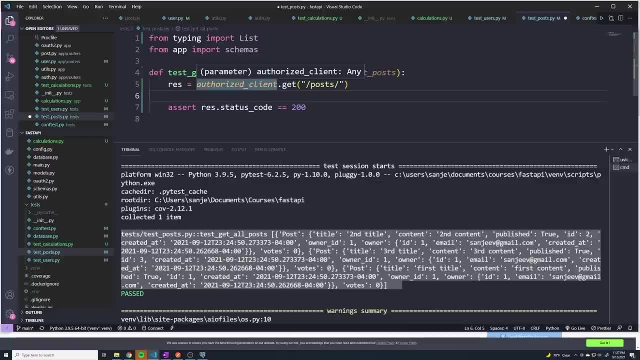 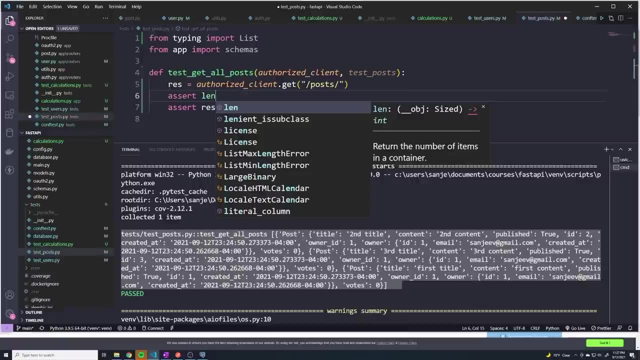 out. If you guys want to take that as a challenge, you can essentially create a post pi dantic model for each entry within within the response and then try to validate each single one. So instead I'm just gonna do a simple check, I'm just going to say assert, and we'll just grab the length of. 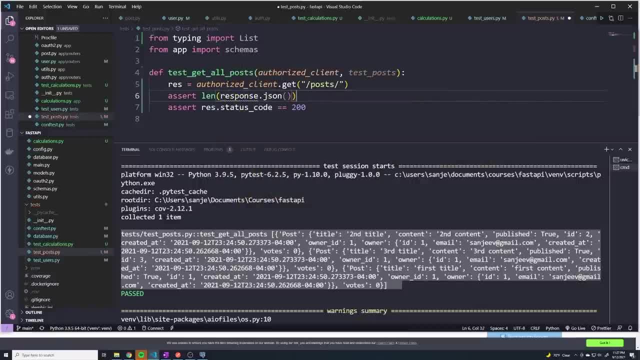 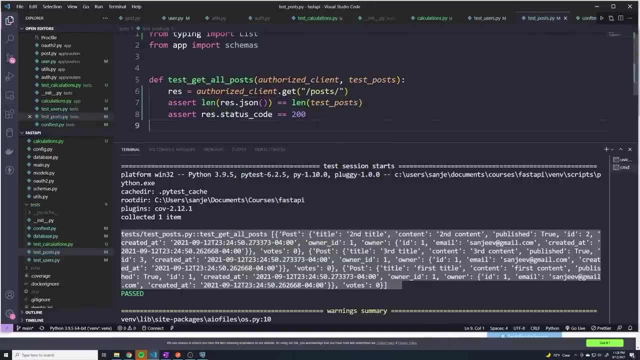 response: dot JSON, And I'm going to set this equal equal to length of test underscore posts just to make sure that we get three exact posts, And if we ever change the number of posts that we have, this should automatically get updated. I think that's a good enough check for this test. 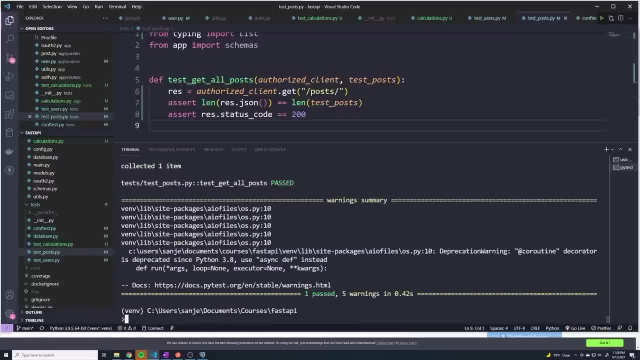 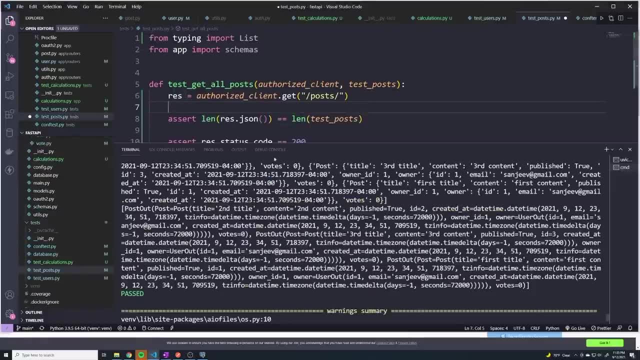 Let's try this again, And we shouldn't get any errors. and it looks like it passed Just fine. Alright, guys. so I figured you know what. let me go ahead and just show you how we can actually do the validation using our schemas. we're going to use the same exact logic that. 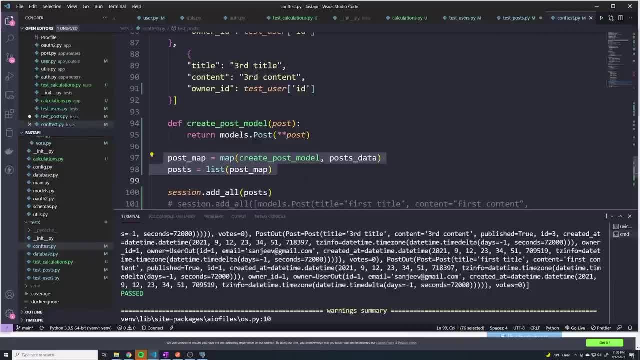 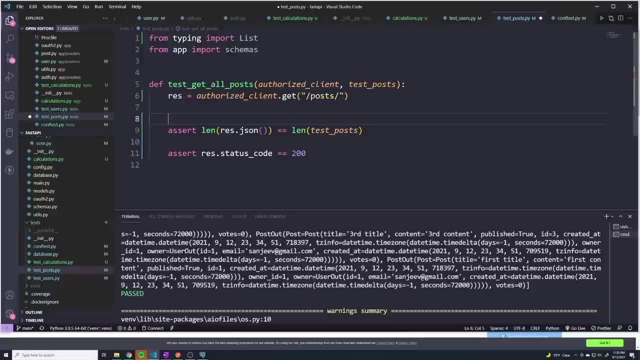 we use here when it comes to performing the map, because we're essentially going to take a list of dictionaries and convert it to a list of schema models. So we're going to go back to our posts, our test, And what we're going to do is we're going to first define a function that's called 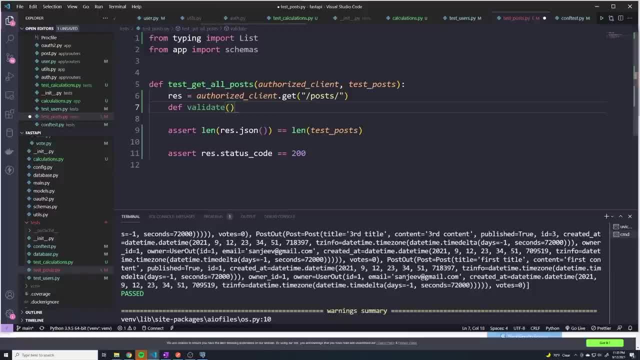 I don't know. we can call it validate And this is going to receive a post And that's going to be a post, that's going to be a dictionary that we get back, And all we're going to do is we're going to return schemas dot, post out. 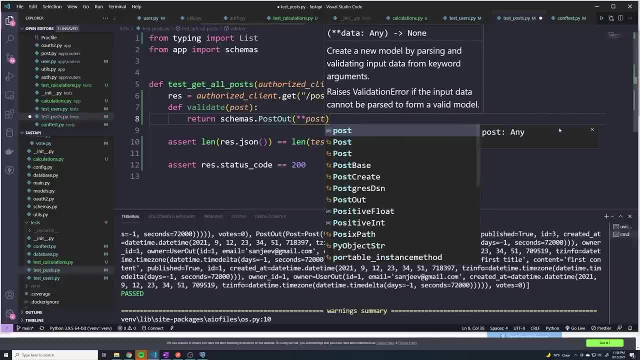 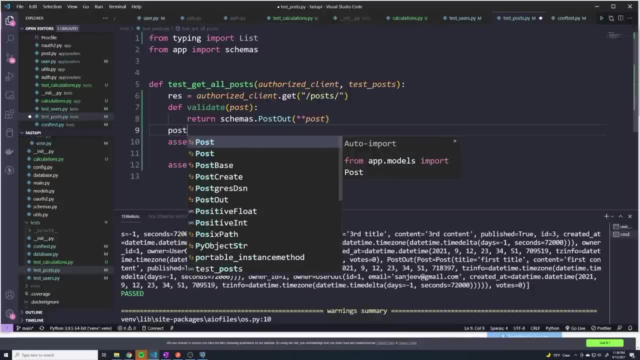 And here we're going to pass in the data. we're just going to unpack it with post. So that's all we have to do. And then we can call the map function, like we did before, And I'll store this in a variable called post- posts underscore map, which equals map. we're 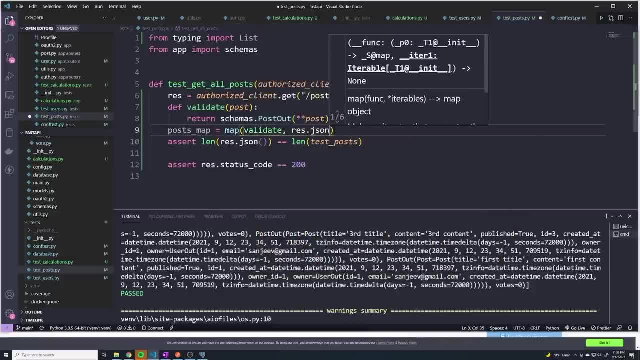 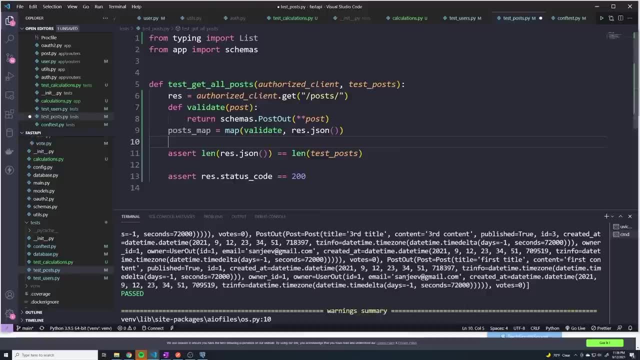 going to call the validate function And we're going to pass in res dot JSON And so we have a map. if you wanted to, you could technically convert it to a list by calling list post dot map, but we're not doing anything with that data. 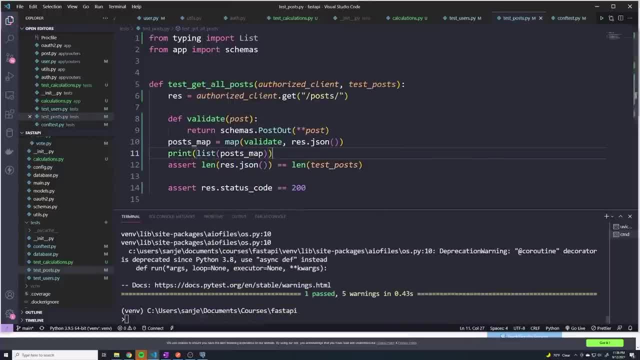 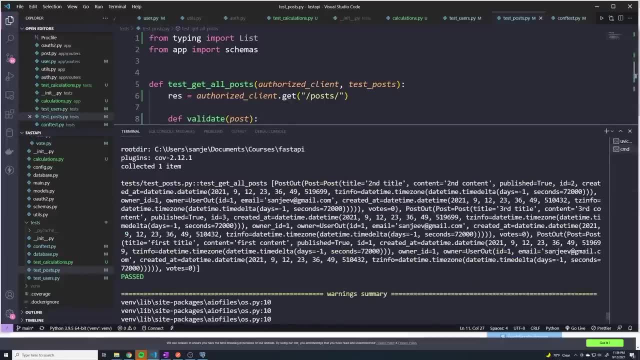 However, just to show you, we can just print this out real quick And so now, if I run this and we take a look at the print statement, you can see we've got a post out model And it does all the validation. 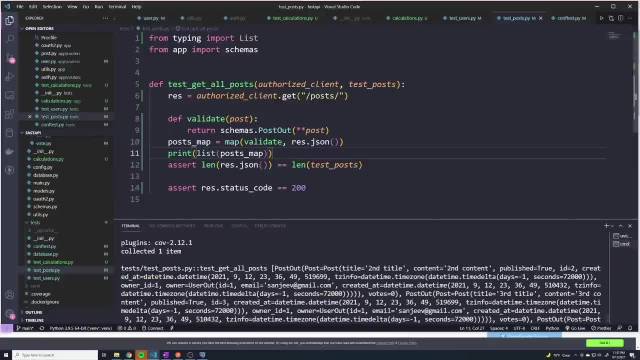 So it's going to make sure all of the properties are set And are there. And because we have it set as a post, as a post out pydantic model, you'll see that it's very easy to perform extra checks with the cert statement. 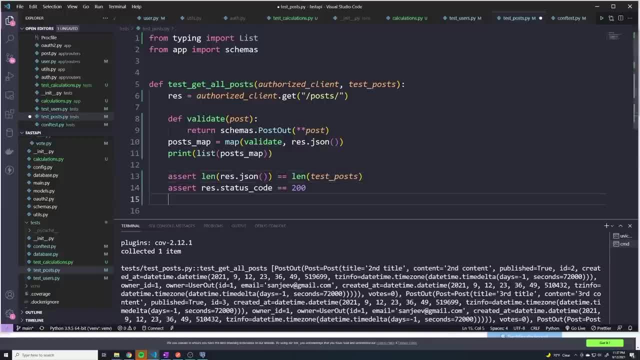 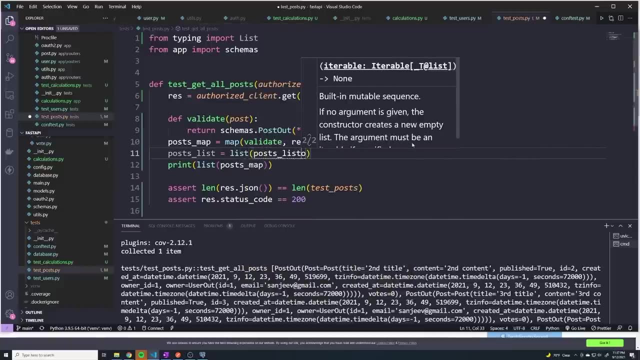 So now I can do other checks, like maybe I want to say actually let me first save this as a variable. say, posts list equals list of posts map. oh, and that's supposed to be posts map. we have access to this list. 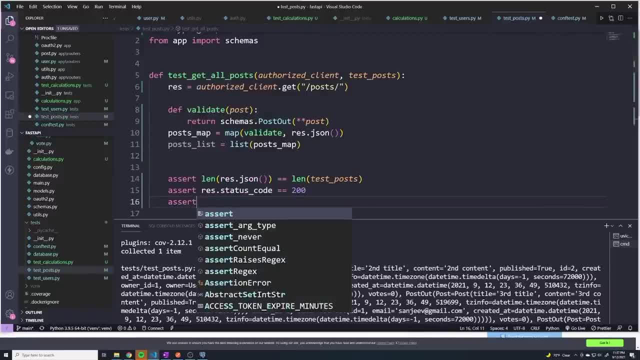 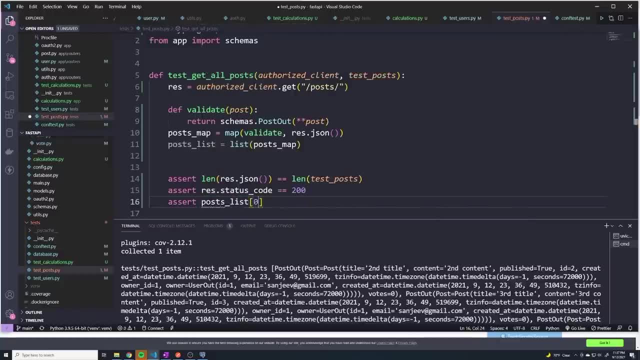 And now what I can do is I can just say assert And here we can grab posts underscore list, grab the first post And we can check certain fields. I can say like hey, does the ID? sorry, it's gonna be. 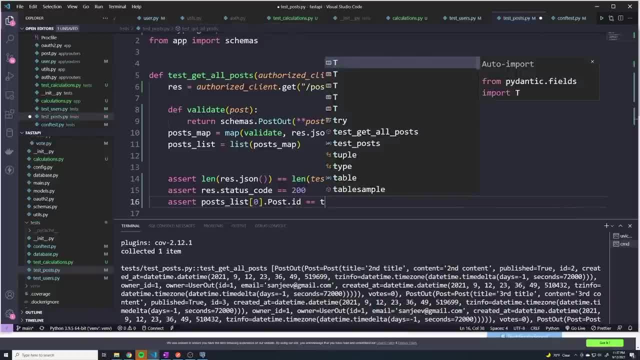 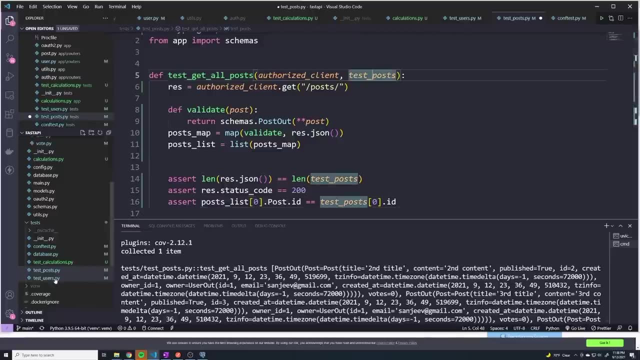 the post dot ID. Does that equal equal test underscore posts. we'll grab the first object And then grab the ID. well, actually it's going to be. I think I could do just dot ID. Yeah, because test post. keep in mind when we do test post, this is going to return. 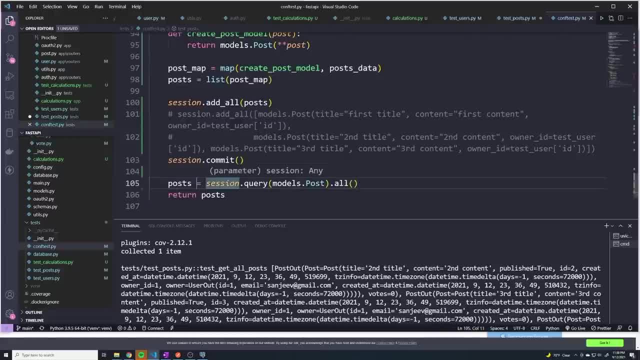 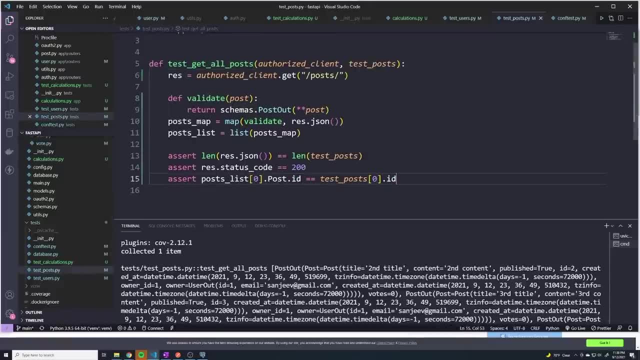 this is going to return a, not a pydantic model or a dictionary, but this is going to return a SQL alchemy model. So a little bit different, But we just call it dot ID And I think this should work. So let's test this out. 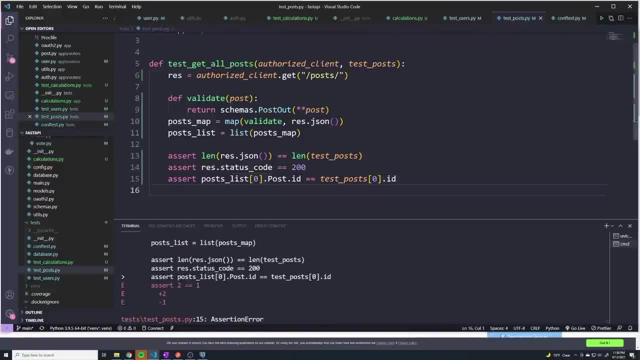 It did not work. What happened here? Yep, So I accidentally grabbed. I see, Yeah, that, So this is expected, just because I don't know the order that we're going to retrieve the posts in. I didn't provide a order by filter criteria. when it comes to my, my get. 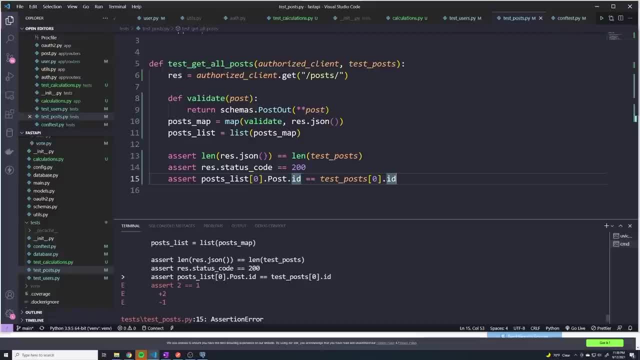 post functionality, So it could be returning any posts. right now it's saying that, hey, this idea happens to be to this, one happens to be one, so it the order doesn't matter, So this isn't exactly the best way to do it. 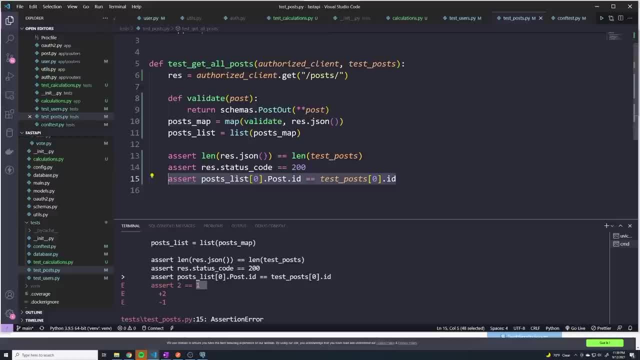 But if you want to Figure out a way to set up the order so that you always receive maybe the post with the lowest ID and then you compare the two, that would be perfectly fine and then you can check other properties like: what's the? the title doesn't match up with what we should. 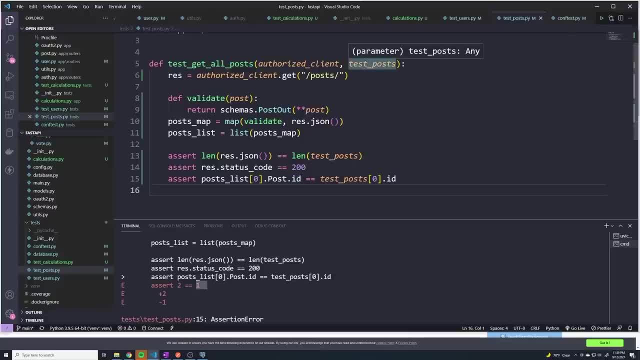 expect it to be? does the content match up with the content? you can put as many asserts as you can, But by having, by doing this, we are able to perform a validation to ensure that at least we get what we expect. All the fields are there, and then it's just up to us to set up the necessary asserts to. 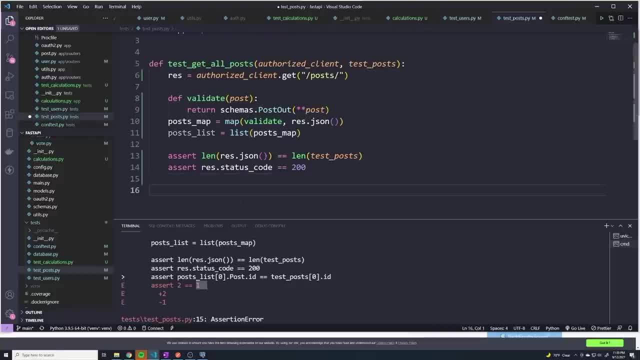 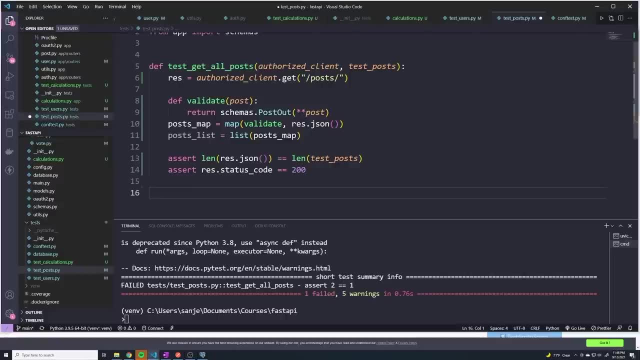 verify that the values are correct. Okay, But I'll remove that and I think it's okay just to keep it like this for now. All right, so we set up a test for getting all posts, And what I want to do now is I want to test to make sure that a unauthenticated user is. 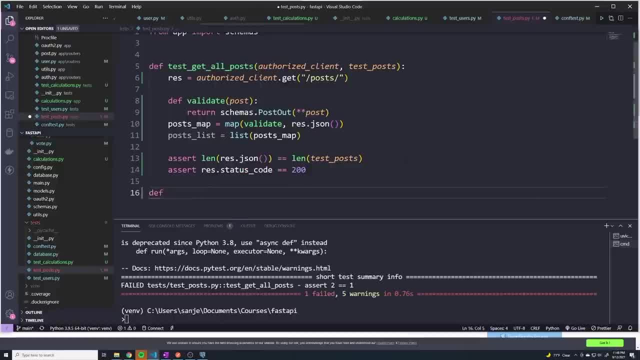 not able to retrieve all the posts, So I'll create a new test and I'll call this test. How about unauthorized user underscore: get underscore all underscore posts And instead of using authorized client because we want to test if a unauthenticated client we want to test if a unauthenticated client gets all the posts. 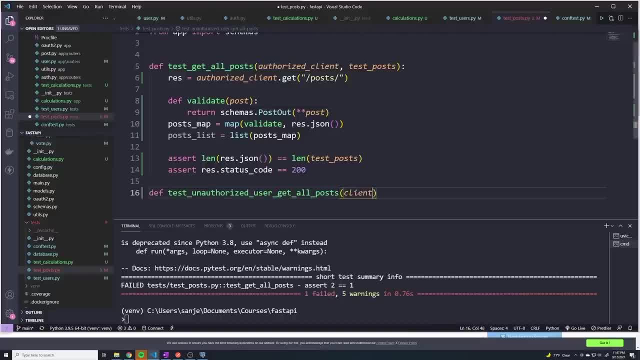 So we can see that we've created a user tries to access as they get a 401, we'll just use the regular client, which is going to be a non logged in user, And we want to make sure that test posts are here as well. 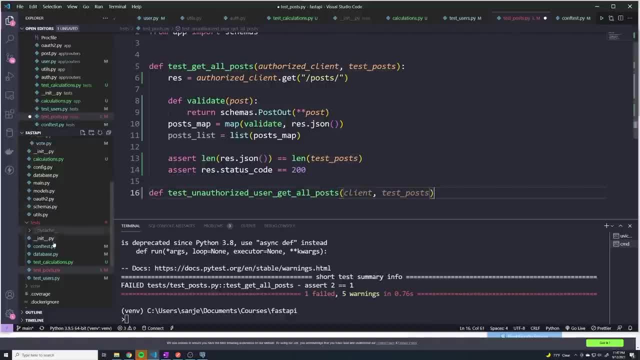 And remember, because we're calling test posts, that's going to ensure that, because test posts is reliant on test user, it will in fact create a test user as well. So, just to give you a heads up, we don't actually have to pass in test user into here, because 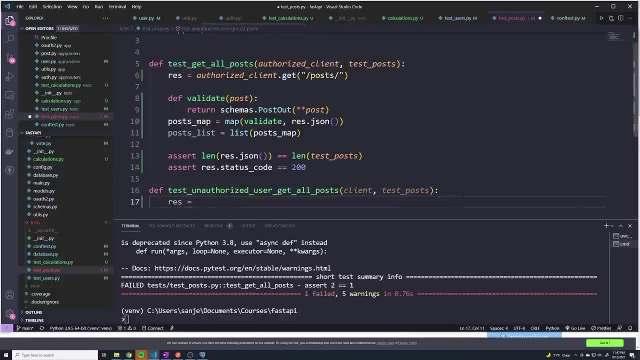 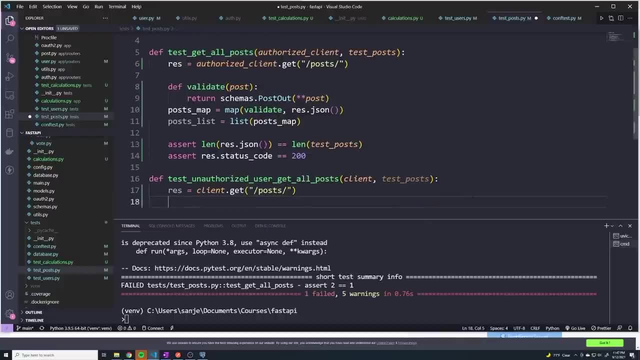 this should handle that automatically. And here I'll just say: res equals client dot. get, And we'll just go to posts again And I'm just going to assert a simple 401.. So res dot status code equals, equals 401.. 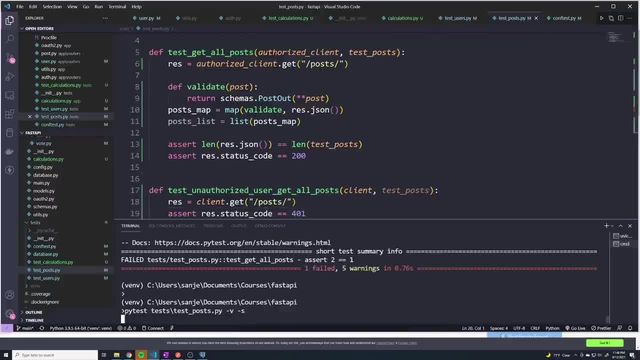 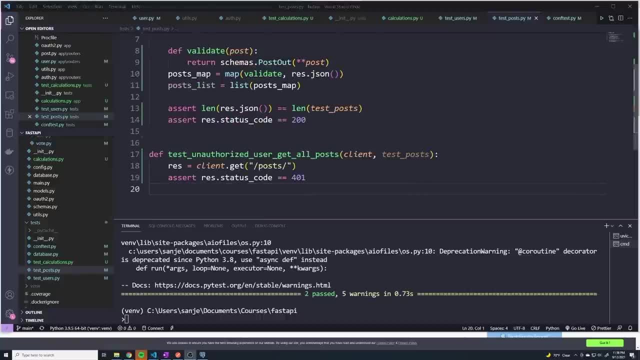 That's really the only check I want to do there. If they're unauthorized or unauthorized, there's no other things to check really- And we can see that it did successfully pass. Okay, so we've tested the get all posts. we're going to now move on to getting an individual. 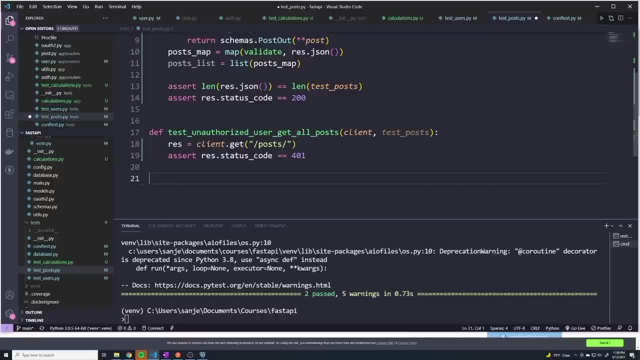 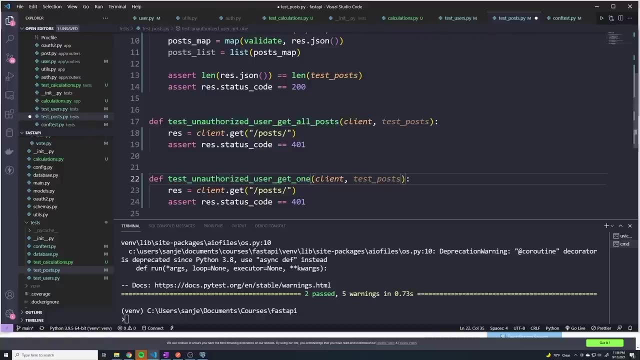 post by an ID. But before we do that, I think it's best to actually test getting an individual post by ID when you're an unauthenticated user, because we can essentially just copy this code And I can just paste it here And instead of doing a user get all posts, this will be user underscore: get one post. 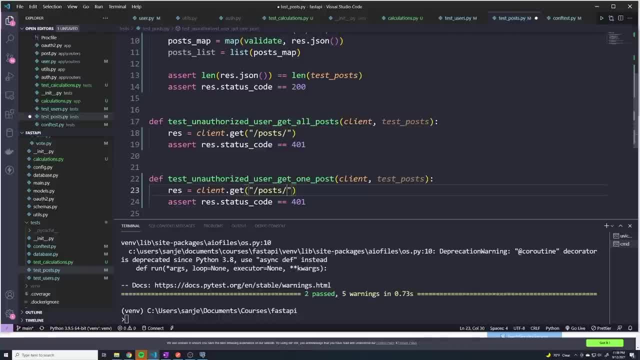 And so everything else can be the same. we just have to change the specific URL, And so in this case we're just going to grab the ID of one of the posts. So here I'm going to change this to an F string. 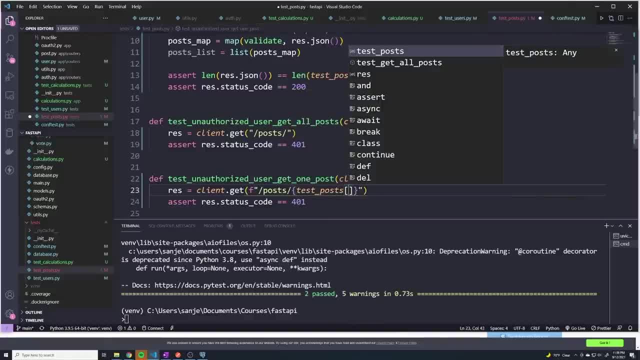 And I'm going to say test underscore posts. I will grab the first one And then remember this is a sequel alchemy model And so we actually have to convert it to a dictionary. So we have to do dot, underscore, underscore, dict, underscore, underscore. sorry, the test. 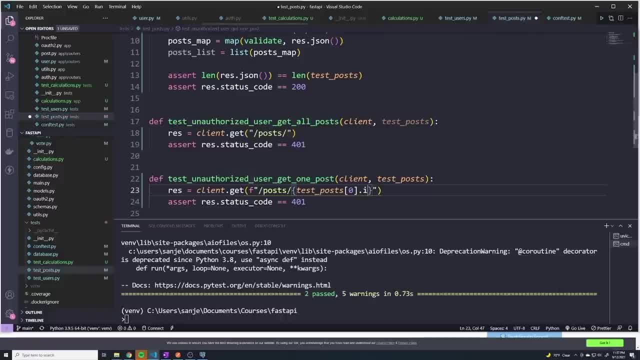 posts is not a sequel. Is it a sequel? I think I could do ID. Okay, I think that should work. Actually, nevermind, I think we should be able to do that. That should be fine And this should be a 401.. 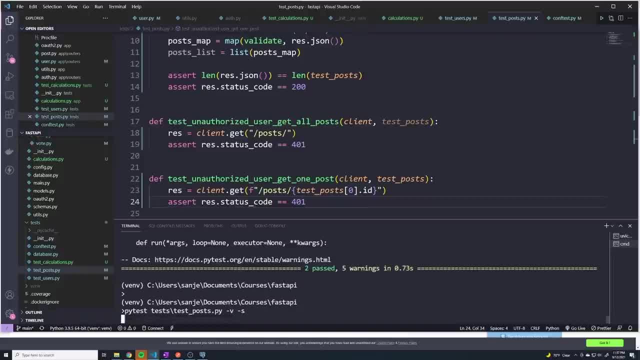 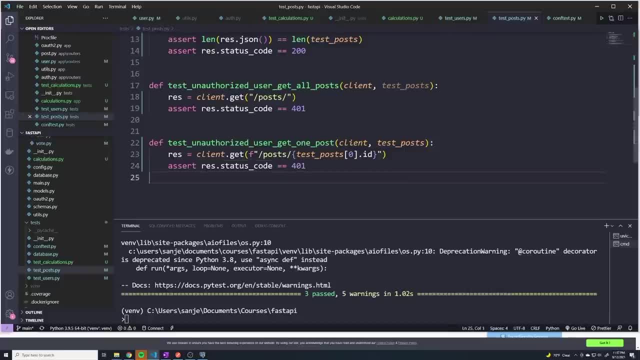 So let's test this out, Let's make sure that this works And that works. And what I also want to do is I want to test for a post, test to retrieve a post with an ID that doesn't exist, I guess. So I'll call this a def test. 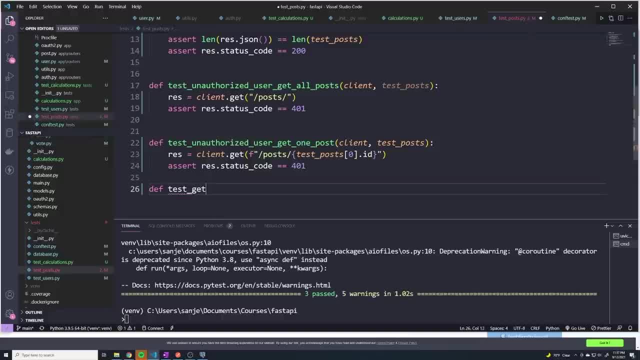 Get one post about not exist, So this one, we're going to need an authorized client And then test underscore posts as well, And I'm going to copy this. But we're going to change this and I'm going to hard code some random number like 888888.. 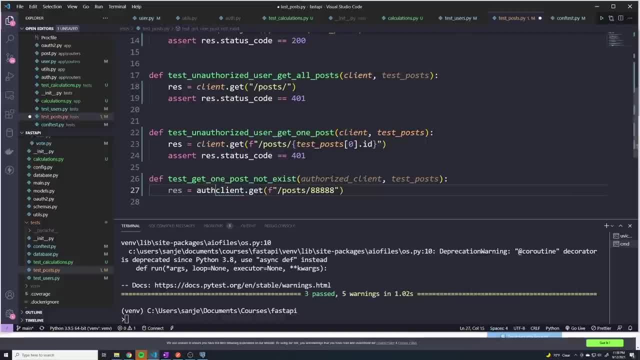 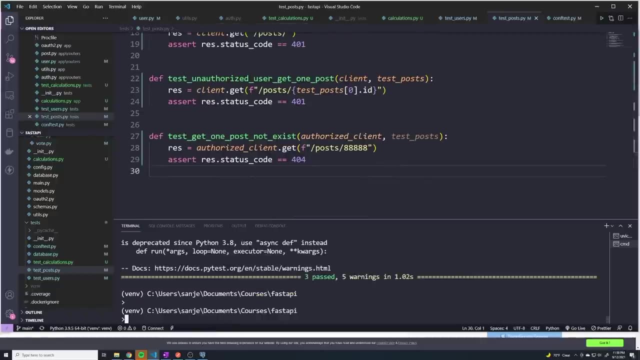 Okay, And then we'll just assert: res dot status. underscore code equals: equals 404.. Alright, so now we're going to try to retrieve a post that doesn't exist And it looks like it passed perfect, So now let's actually try to retrieve a valid post. 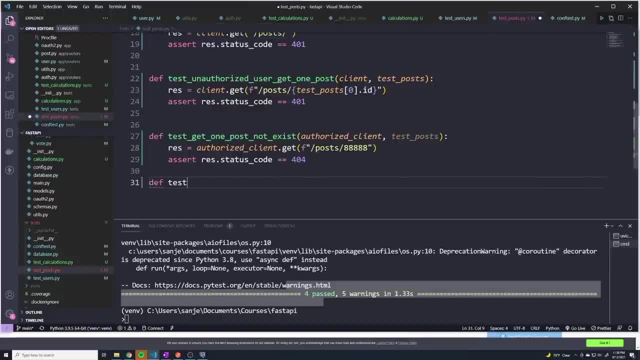 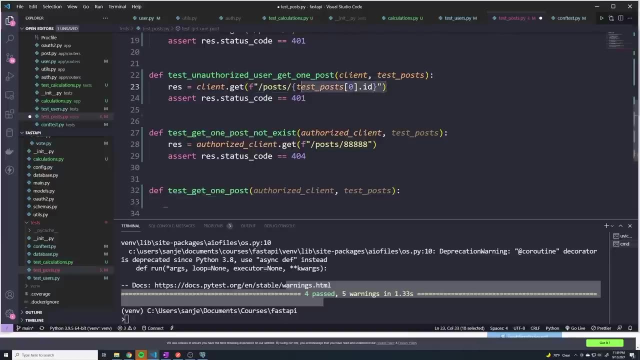 This one's gonna be a little bit more work. So we'll say: def, test, Get one post, And we're going to copy these two And I'm going to copy this one right here. We're going to retrieve the first post from test posts with an ID of zero, I think. 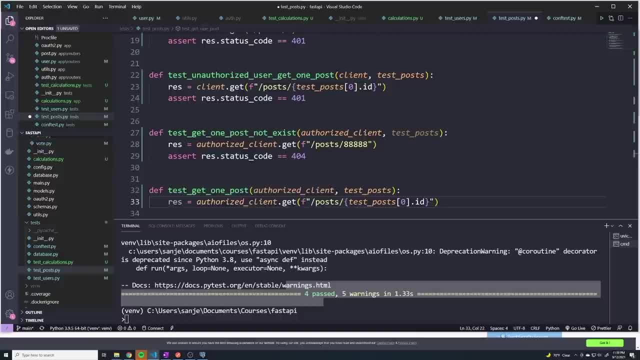 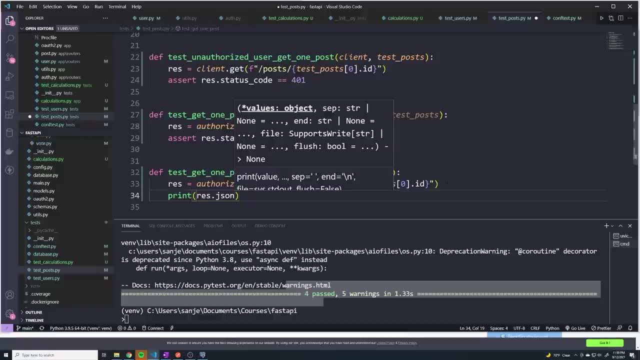 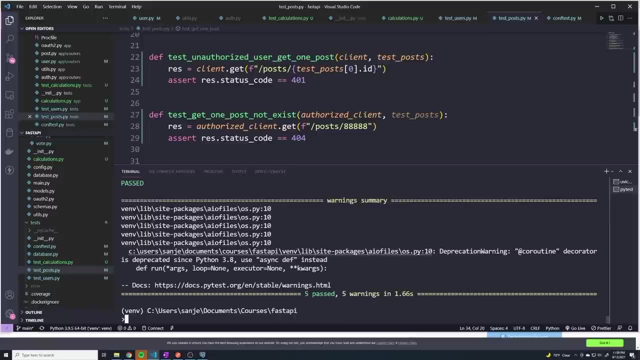 And I'm just going to rename this to authorized client And let's just do this, Let's do a print, Let's see what this looks like. So we'll say res dot JSON, Alright, and that's going to run And it printed out the post so we can see what that looks like. 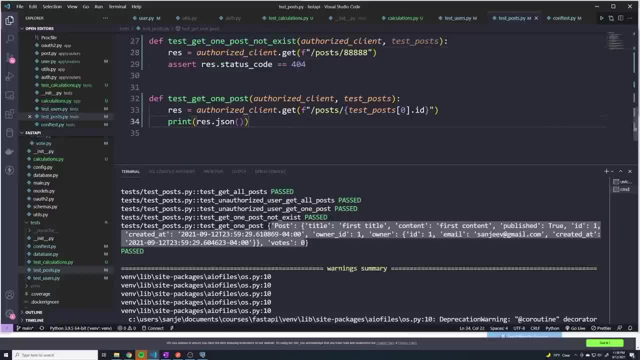 And, just like we did before, we can also do a validation. So I can say: post equals schema, Schema's dot. what is it? I think it's post out. Yeah, post out, And we're going to pass in res dot JSON. 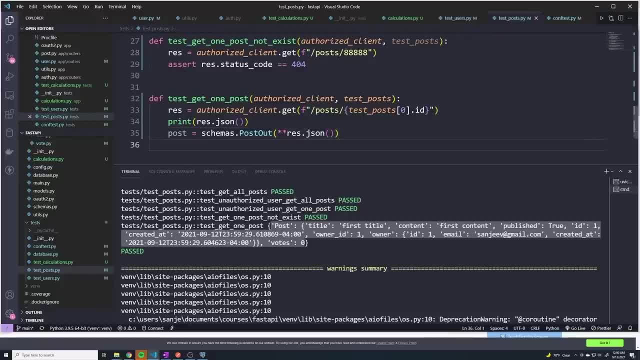 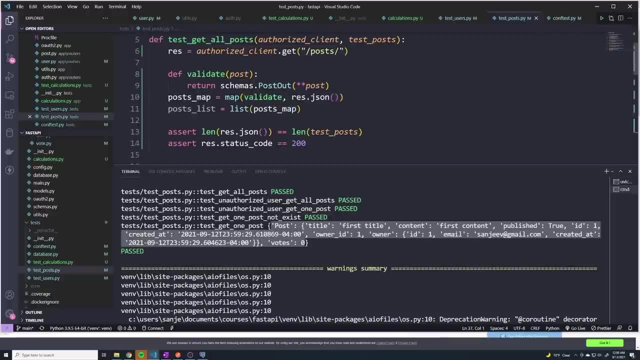 And do we need to unpack it? I think we have to unpack it. Let me print out post just to see what that looks like. Actually, I could just take a look at what we did up here. Yeah, we have to unpack it. 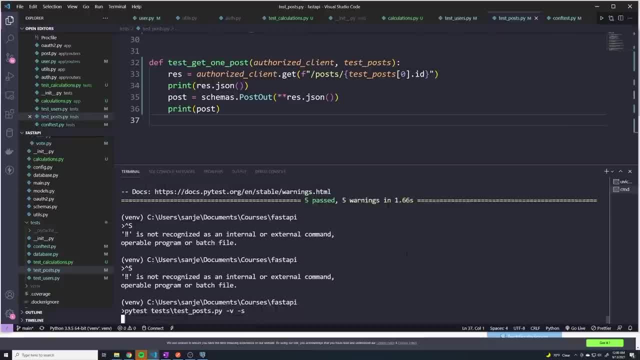 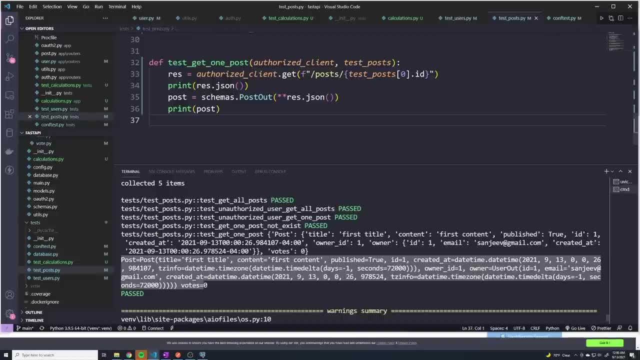 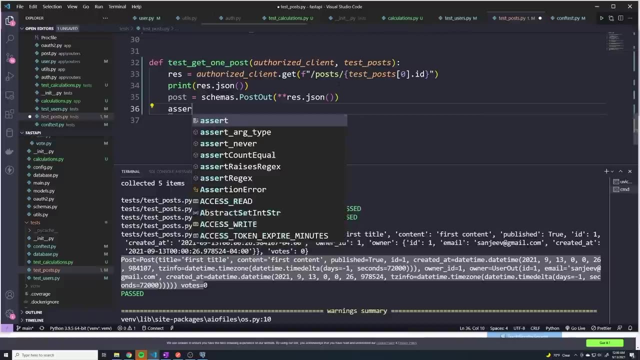 Or spread it whatever it's called. Okay, Yep, so now we've got our post model. Well, it's our pydantic model, And so that does some level of validation. And then at this point, what we can do is I can say assert. 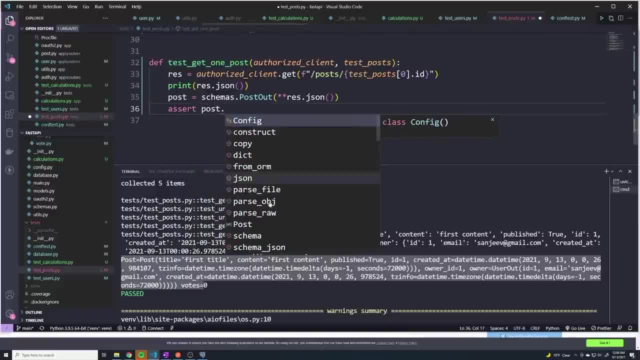 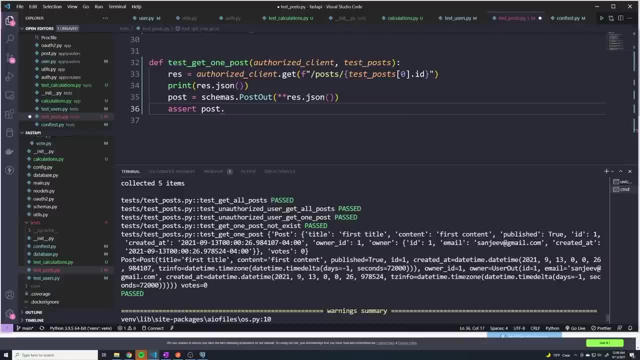 And I could say: does post dot? And then take a look at the format. We have to grab the post property. Actually, it's this first one, Yeah, So we'll grab post dot. post dot ID equals equals. then we're going to compare it to. 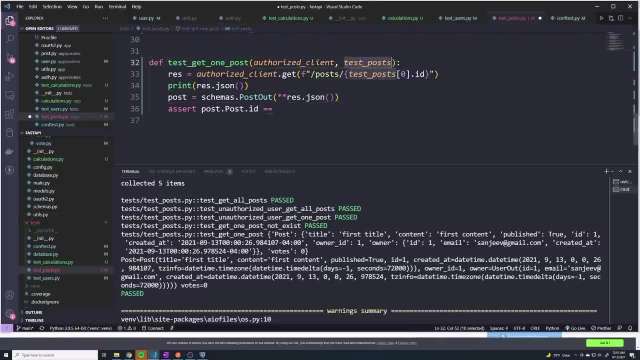 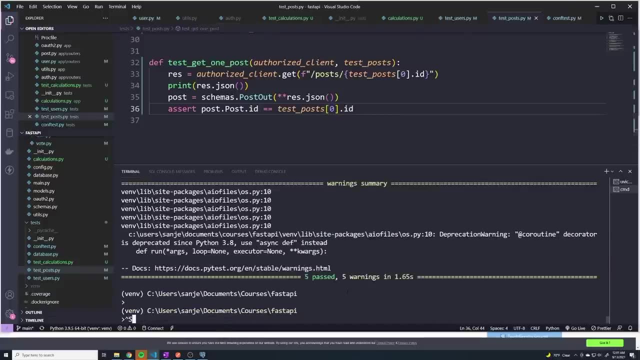 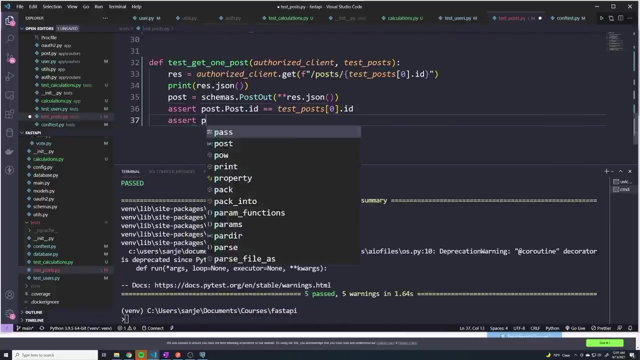 the ID from test underscore posts. So it's a test underscore posts, zero dot ID, And I think that should still work. All right, that works, And we can check a few other things. So we can say: post dot, post, dot, content. 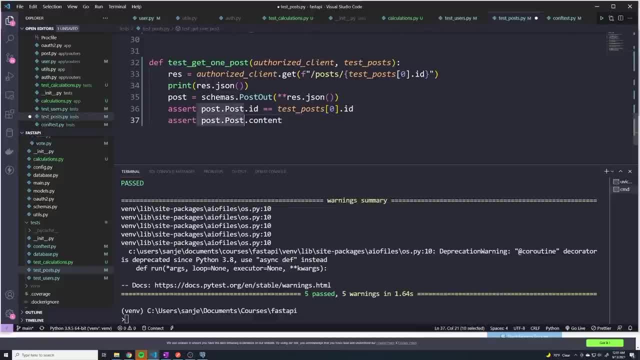 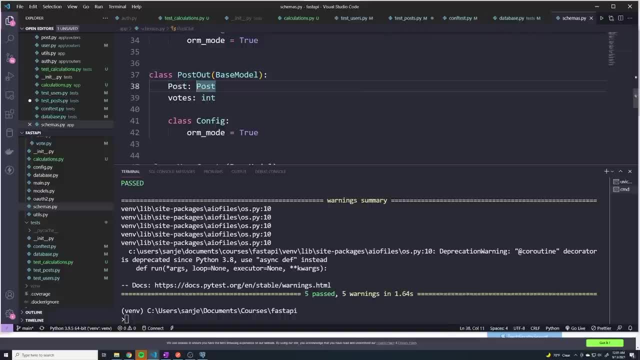 And if you're wondering why it's post dot post, remember, if you actually take a look at our schemas, our post out, you can see that we have to grab the information about the post. we have to go into the post property. 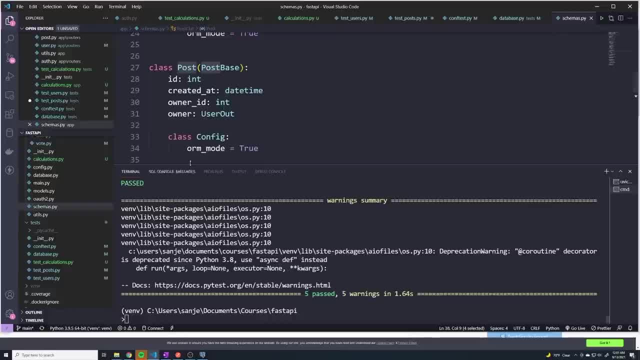 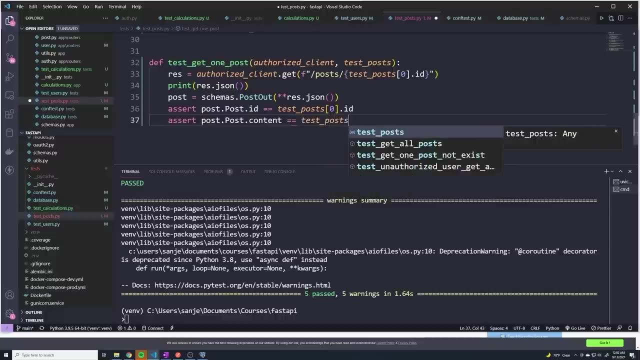 And then from in there we can then take a look at all of these fields. So that's why we have to do it. So that's why we have to do it like that And we'll say: test underscore, posts Zero, and then let's see if we can do content. I believe this will actually throw an error. 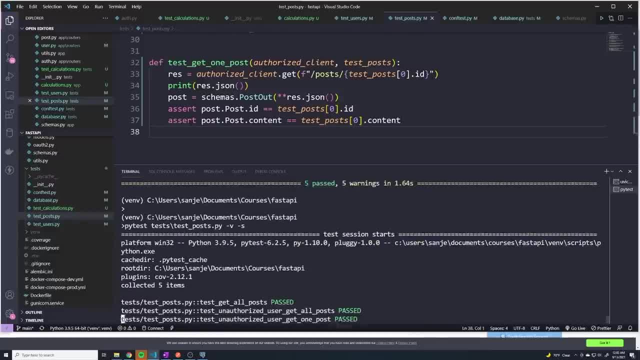 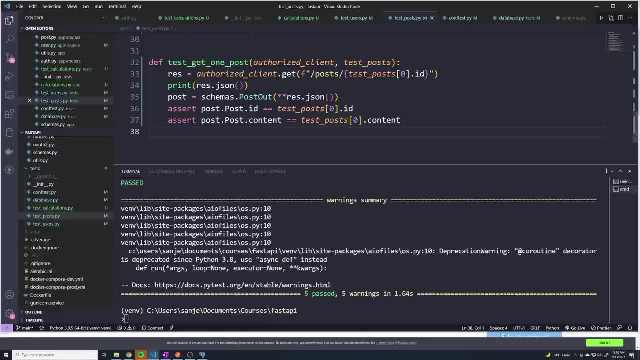 Because this is a SQL alchemy model, So it's going to: oh, that actually did work. I'm surprised. Okay, All right, that worked. So if you guys want to, you can also essentially copy this line and then check to see if the 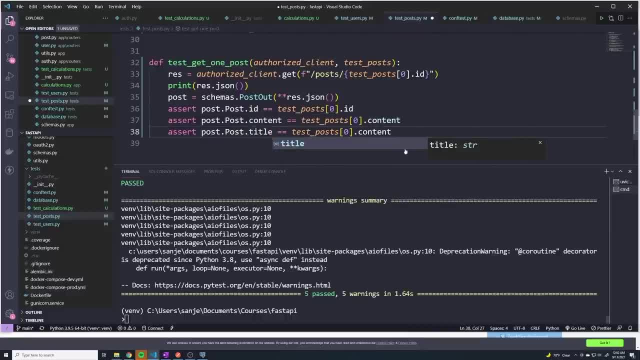 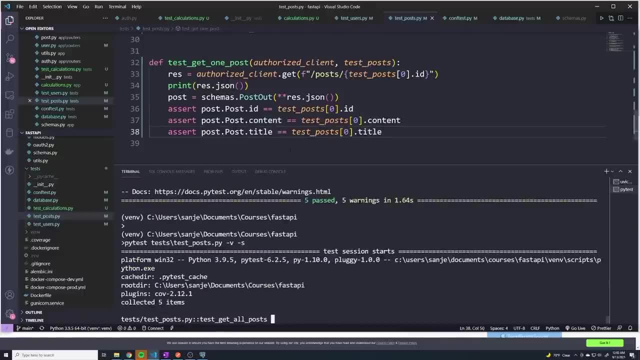 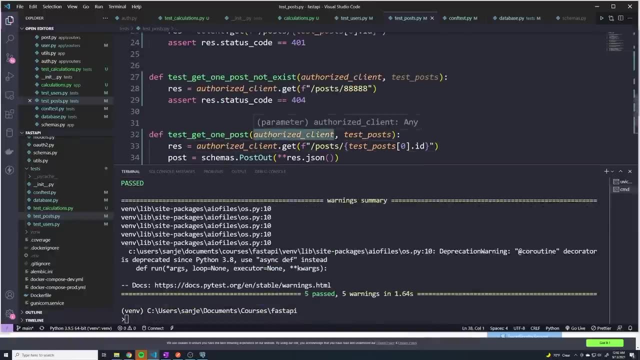 titles match, You can essentially check every property if you really want to. So we'll just run that one last time. Perfect, And I'm just going to remove this print statement. And so those are all of the tests that I want to do when it comes to retrieving an individual. 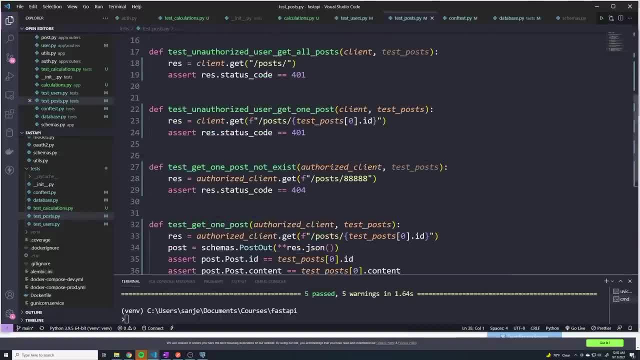 post. I think I'm sure there's a couple of tests you guys might be able to think of, so feel free to implement that. That's a good starting point on this, But in the next video we'll take a look at creating a post. 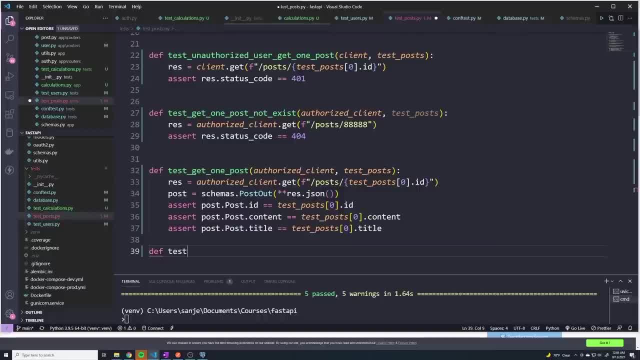 Okay, so let's move on to creating a post. I'll create a function, we'll call this test create post, And we're going to need an authorized client, we're going to need a test user, for sure. And lastly, this is purely optional. 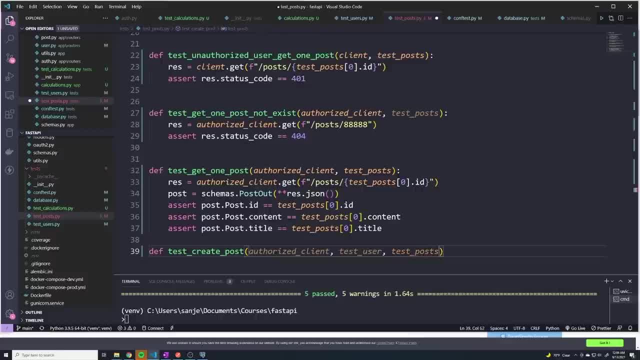 If you want to, we could also set up all of our test posts if you wanted some posts in the database before you created one, just to potentially see if you run into any issues when it comes to creating posts. And there's already posts, but it's optional. 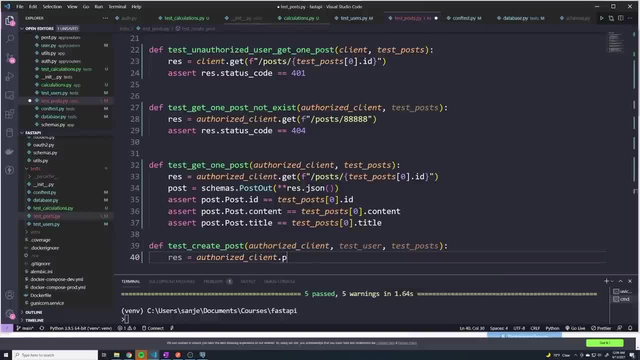 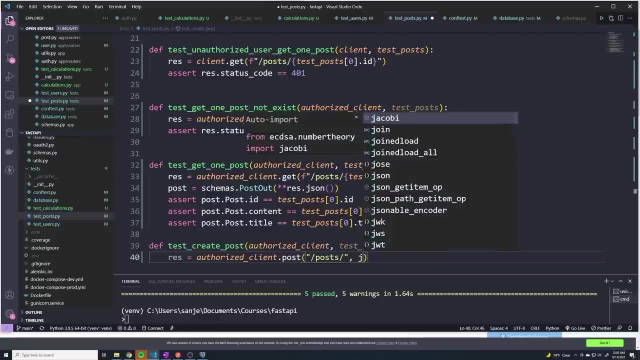 And we're going to set the res and we'll set this to authorized client dot post And the URL is going to be slash posts And then let's give all of the data for our new post. So we'll say JSON equals title. 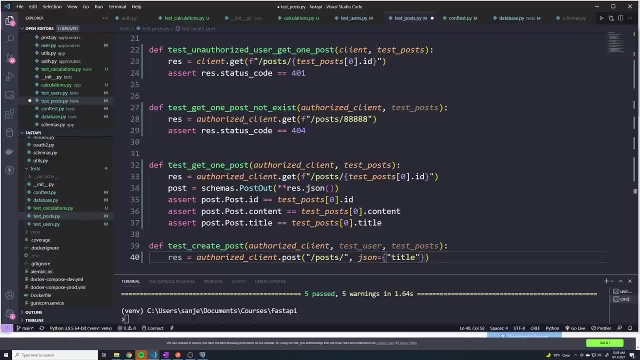 And you know what, instead of doing this, let's go ahead and set up a Python. Let's go ahead and set up a Python. Okay, So we'll say PyTest dot, what was it called? I already forgot what it's. what do we call? 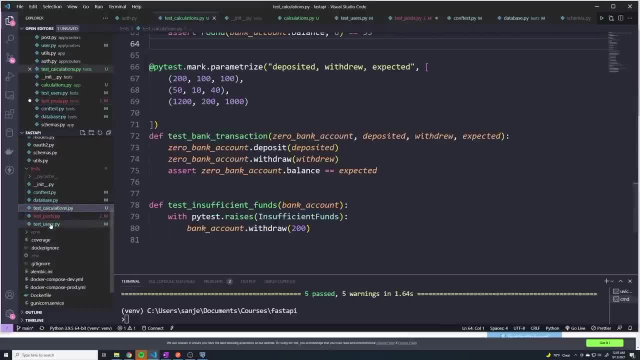 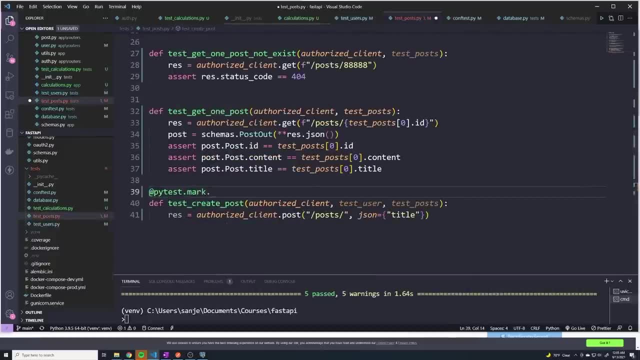 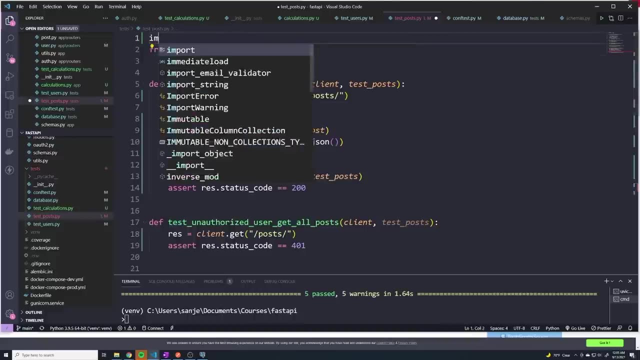 it a parameterize, So mark parameterize, so that we can test multiple different values. Mark dot. why is that not working? Okay, I have to import PyTest. We don't need this line right here, So we'll say import PyTest. 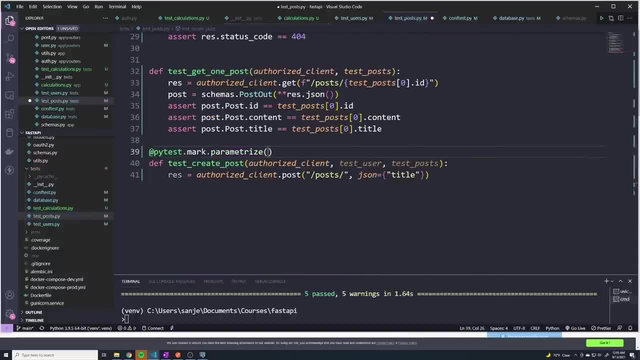 Okay, All right, And so what are the values that we need? How about title? We need title, for sure. We need content, And then we can also give a published value if we wanted to. And then let's give all of our come on VS code. 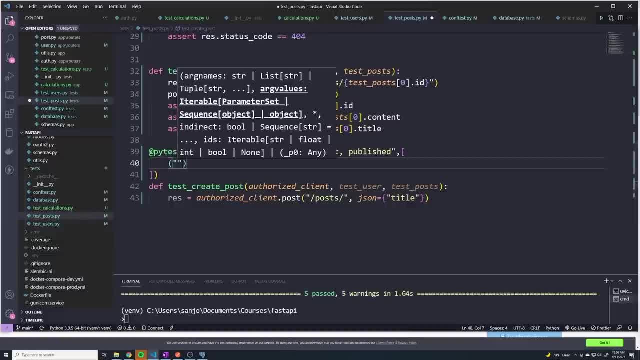 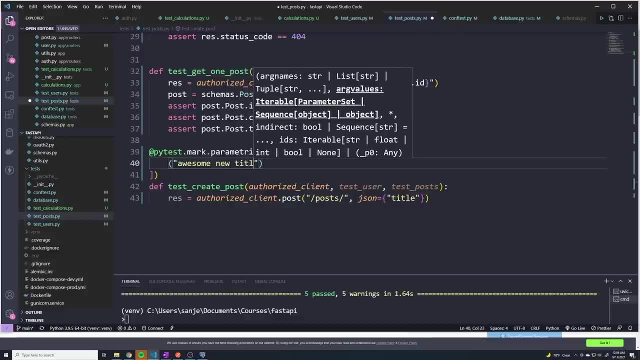 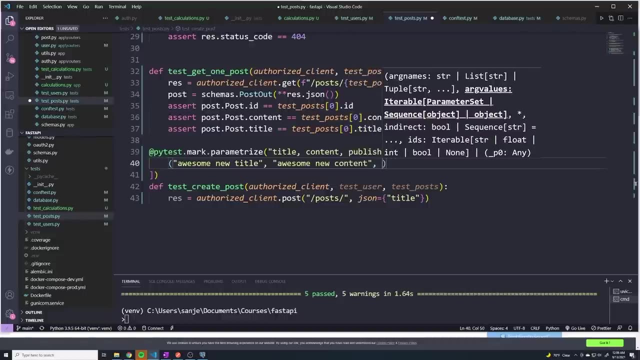 Don't do that. All right, First tuple, What do we want? the title? How about awesome new title. Ooh, Awesome new title. What's the content? Awesome new content. And what do we want published to be? How about true? 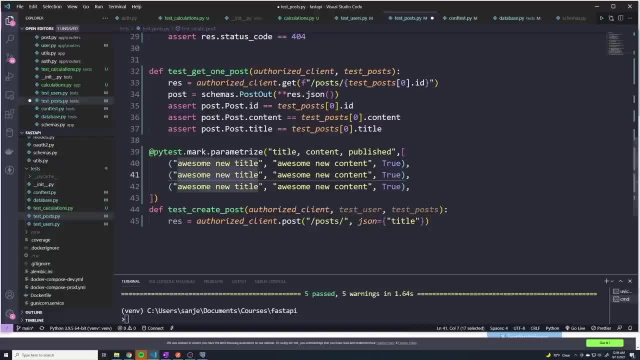 And we're going to copy this and I'm just going to put in some new values: Favorite pizza, And we'll see. I love pepperoni- Ooh, Published. Let's see, That's still a work in progress, All this skyscrapers. 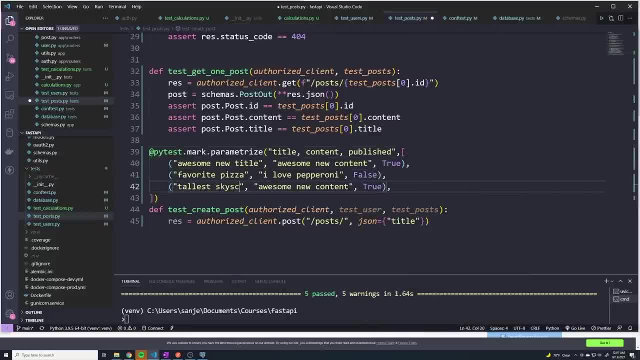 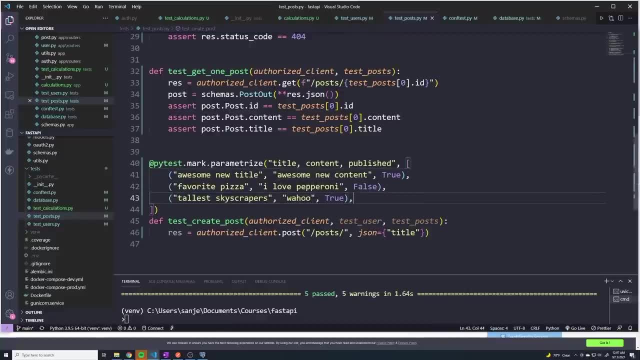 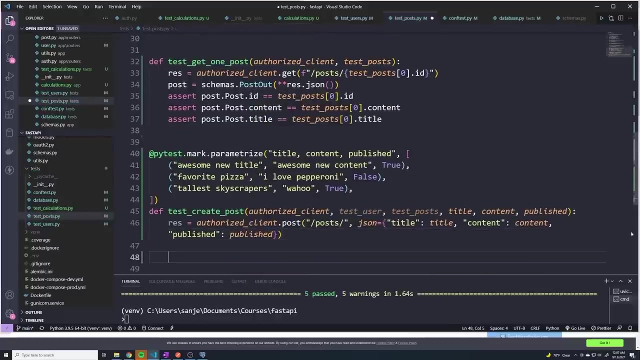 All right, So we've got some test data, Let's pass those values in. All right, So we've got some test data. So title: it's going to be set to title, content is going to be set to content And then, finally, published will be set to published. All right, we get a response back. 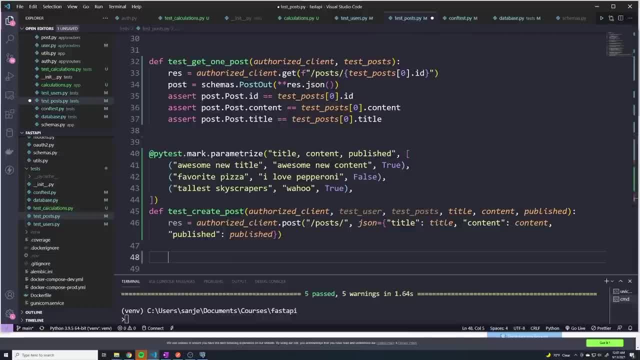 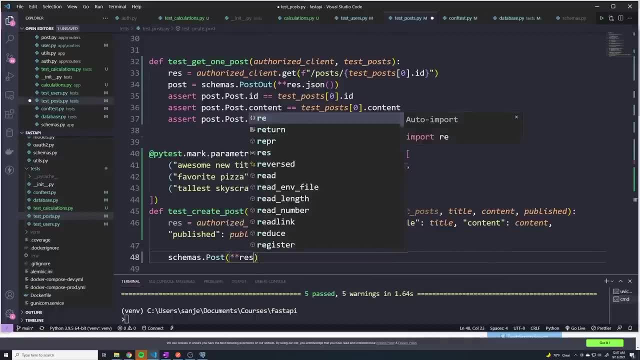 Let's do a little bit of validation with our pydantic model, So I can say schemas dot post, And we'll just take the response, convert it to JSON, of course, and set that to created underscore post, And then we can just run a couple of checks. 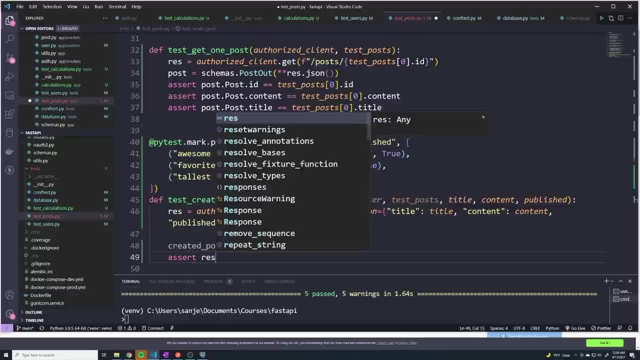 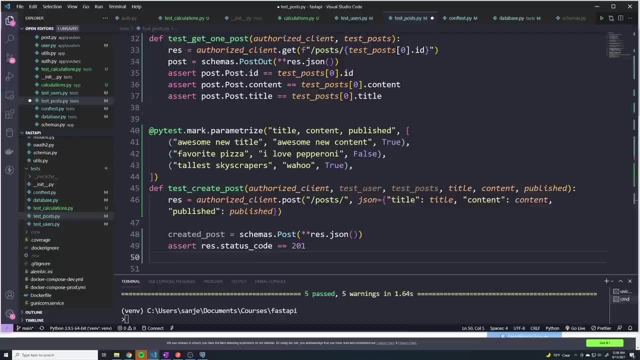 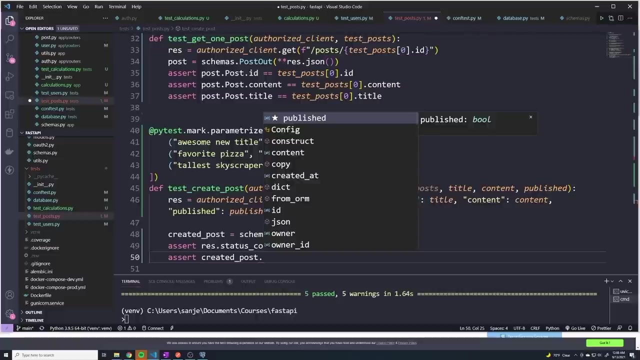 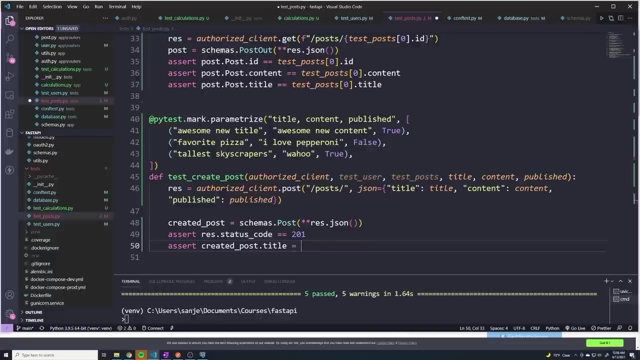 So let's assert the status code, So for creating a new post, that should be a 201.. And then for we can just assert a few extra values So I could say, like res dot, I can grab created underscore post dot. title should equal title. 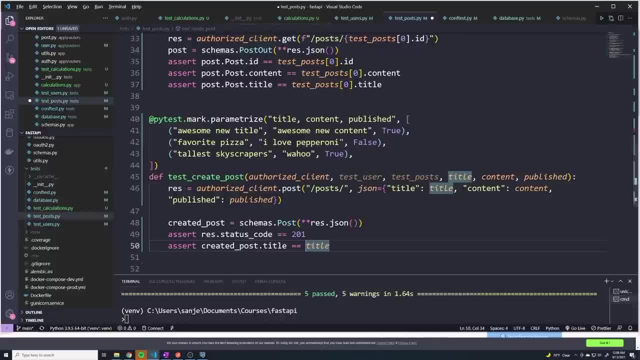 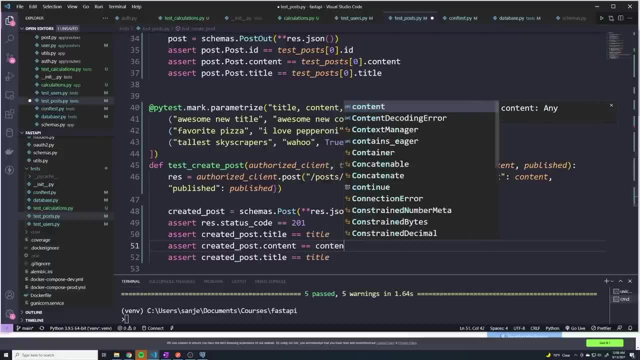 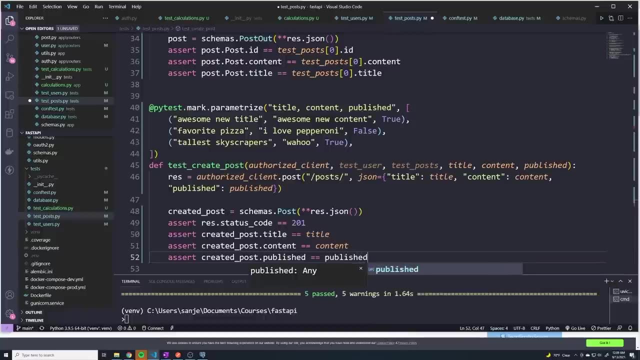 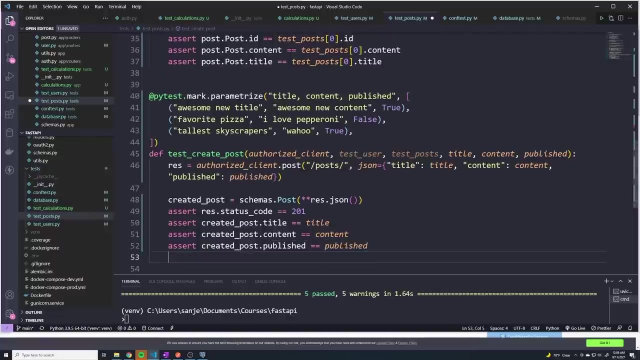 And I can just do that. I need two equals, And then I can just copy this a few times: we'll change this to content, content and then published. And while we're at it, we can also verify that the owner ID gets set, so I can say created. 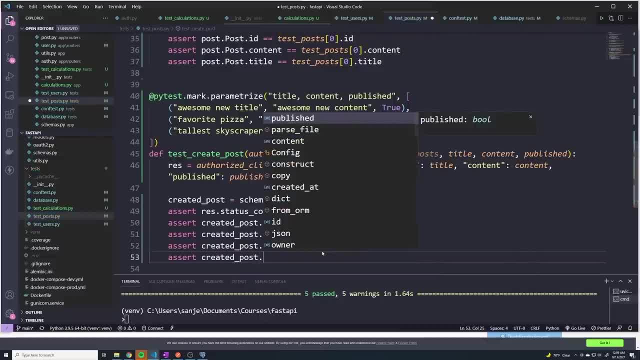 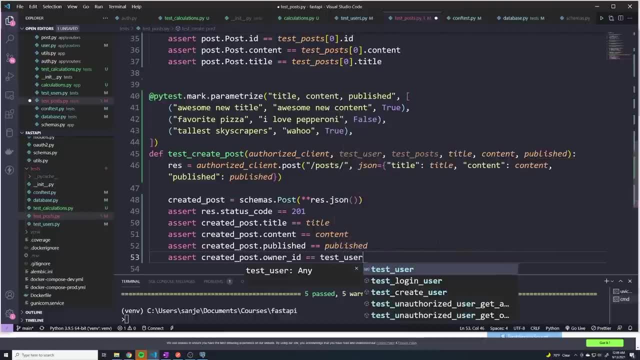 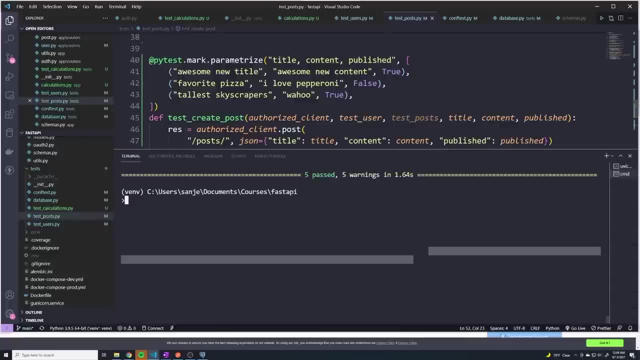 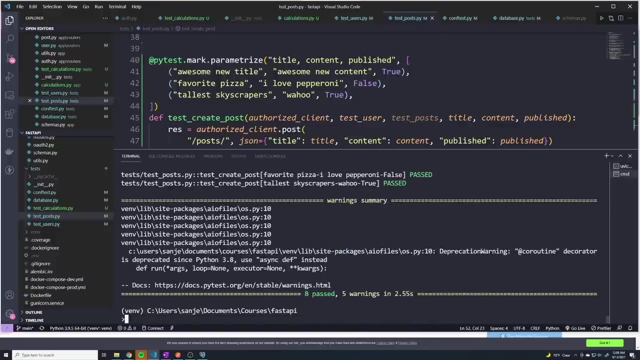 underscore post, post dot. owner. underscore: ID equals equals, and then we can grab a test user ID. So I think that's a good number of things to check. At this point, I think it's safe to say that all of these should work. 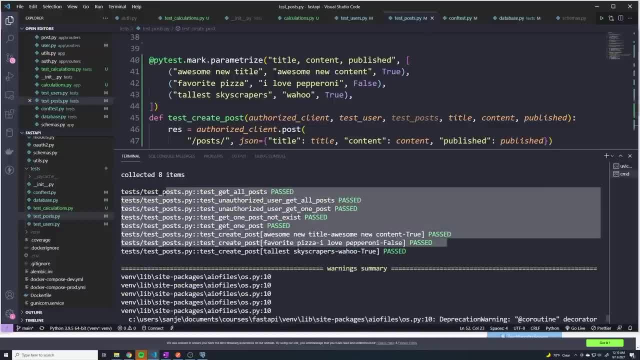 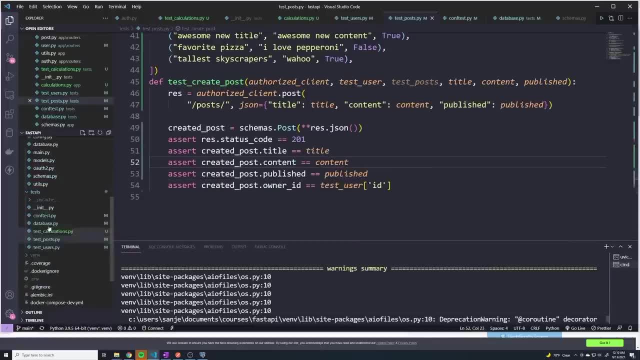 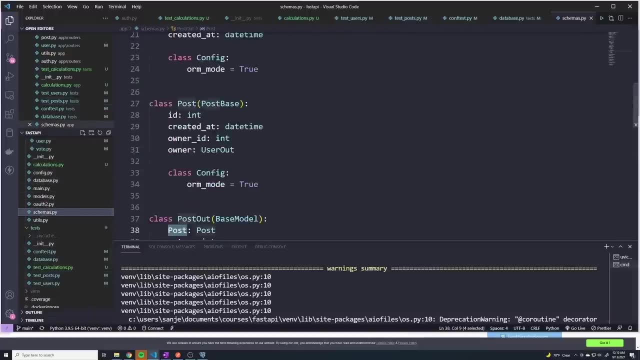 And all of those past Awesome. So we've got the create post done. There's one other thing that I want to test with create post, Because if you go back to our what is it our schemas? where's our schema? I don't know if we have a create post, post create. 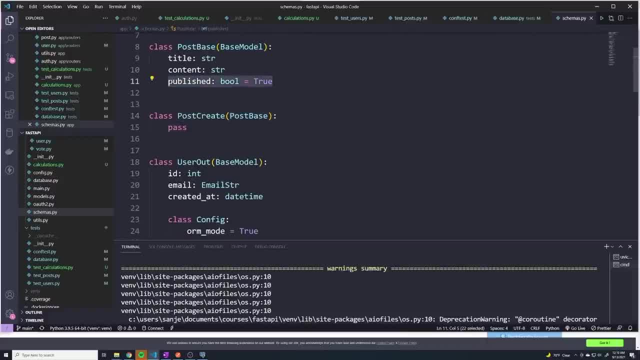 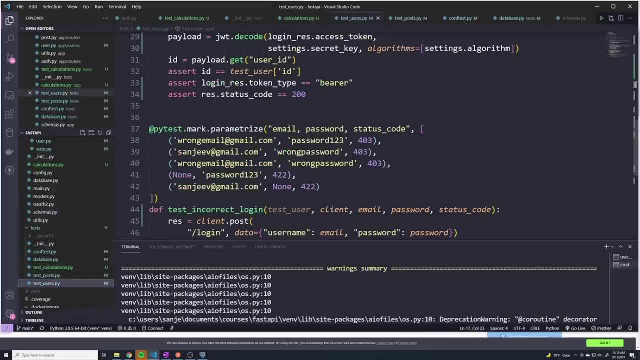 So that's just going to be from post base. we can see published is set to a default value of true. So let's test to see if the default value of true gets set. And we theoretically could have put this test in here just by doing a none here. but I like 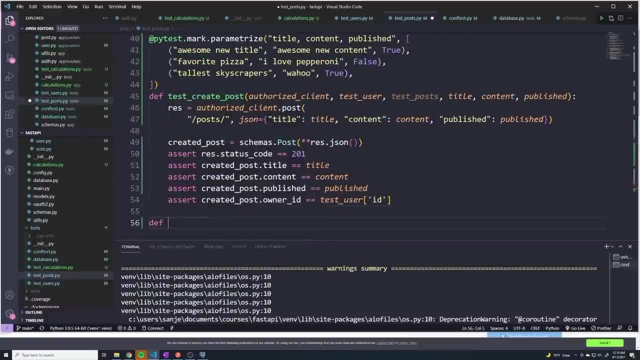 to separate this out. So we're going to do a different test because we are testing a different functionality in this case. So we'll say test, create post, default published. true, I'll do authorized underscore client and test user. Once again, we don't need test posts. 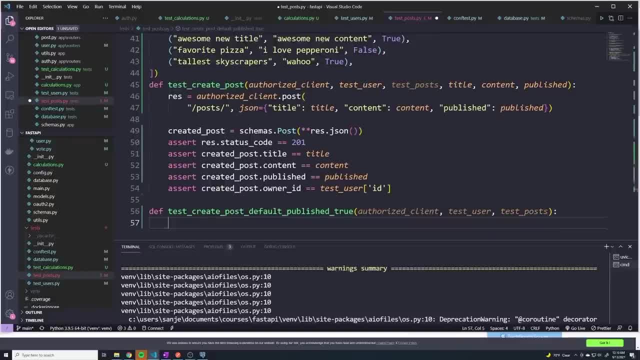 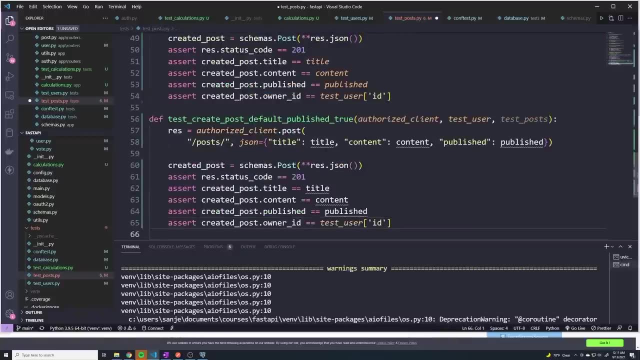 But if you want to have it in the database, just to make sure that everything's not broken when you already have posts already in there, we can keep that in, And I'm just going to copy this. Actually, I can essentially copy all of this. 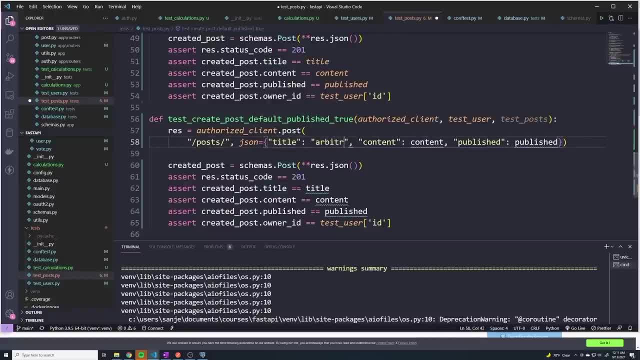 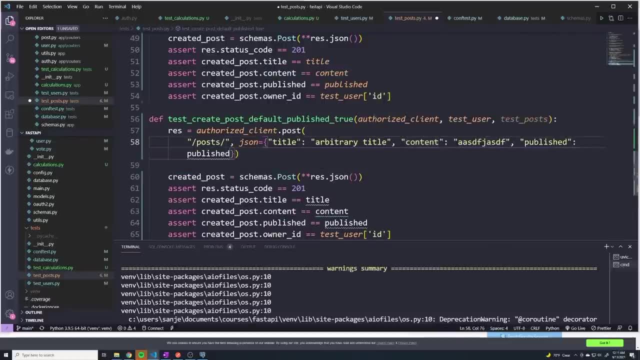 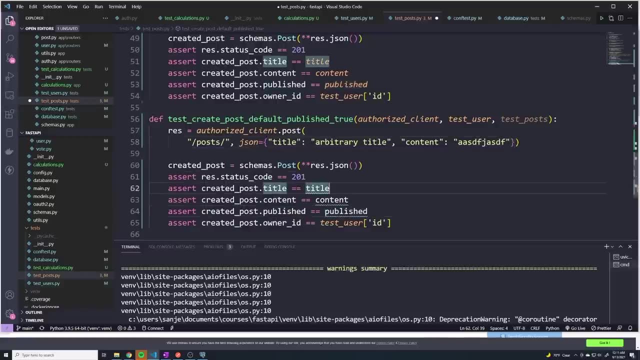 And we can just give it arbitrary titles And then published. we'll leave out published. we don't want that anymore And I'll just copy these values here. And published should be set to true by default. So even though we're not passing it, it should get set and everything else should still. 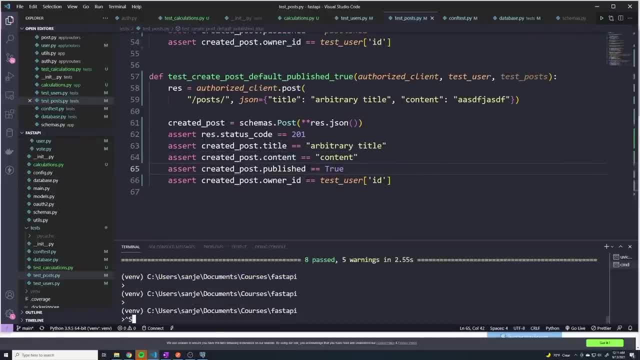 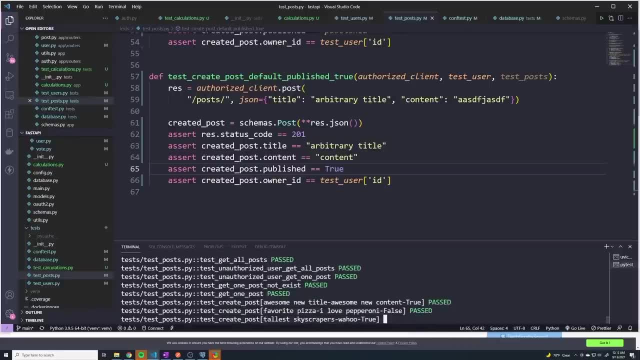 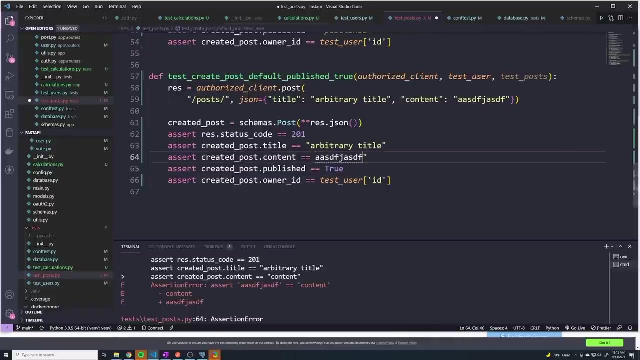 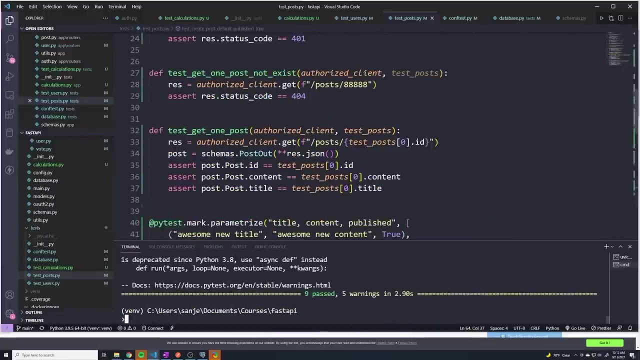 be just fine. So let's test that out. Oh, it looks like it failed. So what happened here? Oh, I just pasted in the wrong values, All right. and then one last thing, just like we did for all the other routes within the. 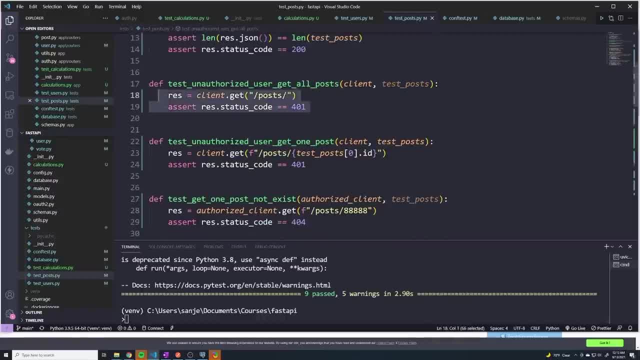 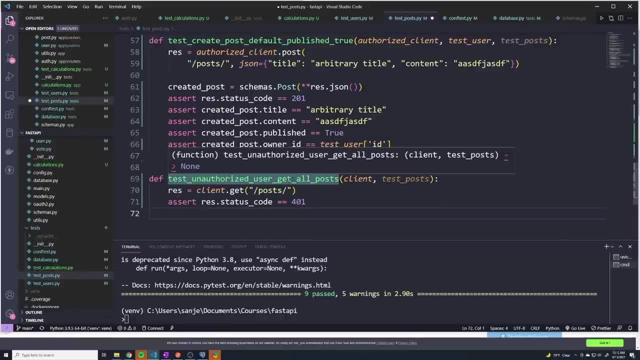 post. we also want to test if we're not logged in, So I'm going to copy this one And just rename it. So: test unauthorized user, Create post. we don't need to have test user in there, but why not? 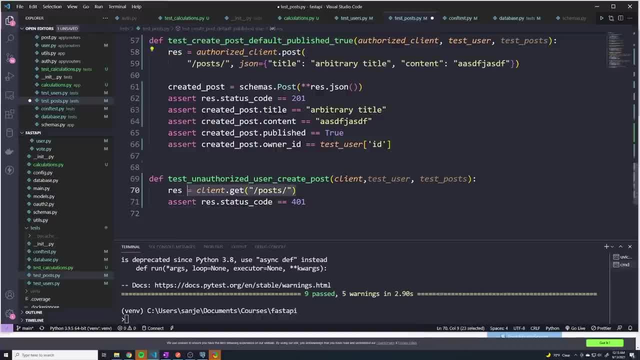 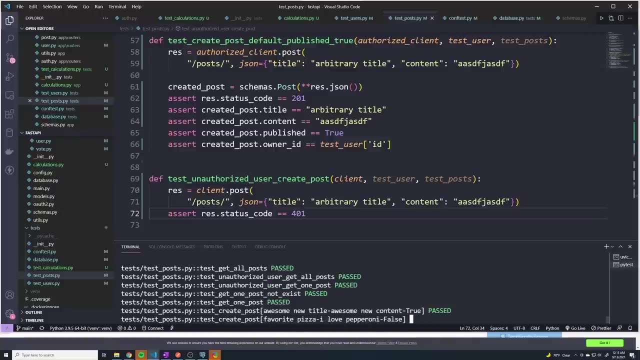 And I'm going to just copy this right here And then just change this to a plain client: All right, And this should Work. All right, and that passed as well. So we have got all of the create post tests done. 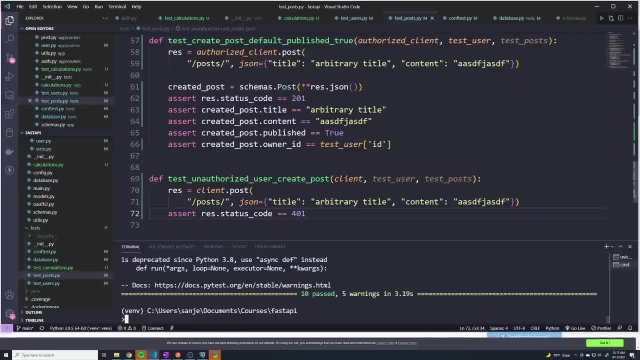 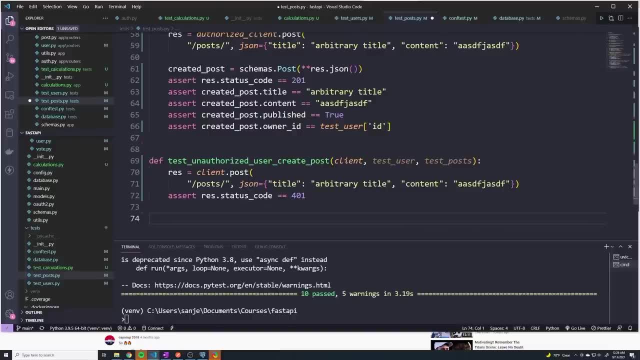 I think in the next video we will tackle either deleting or updating a post. Okay, so let's move on to deleting posts, And the first thing that we're going to do is we're going to test a unauthorized user trying to delete a post. 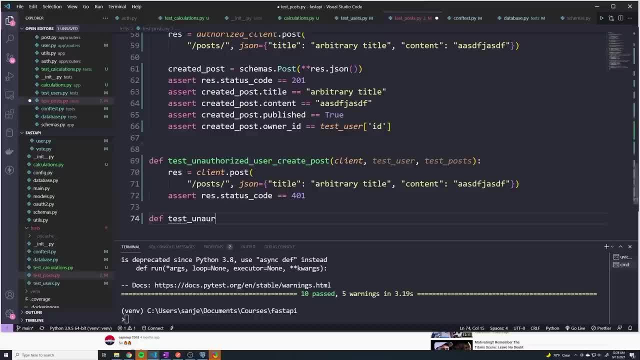 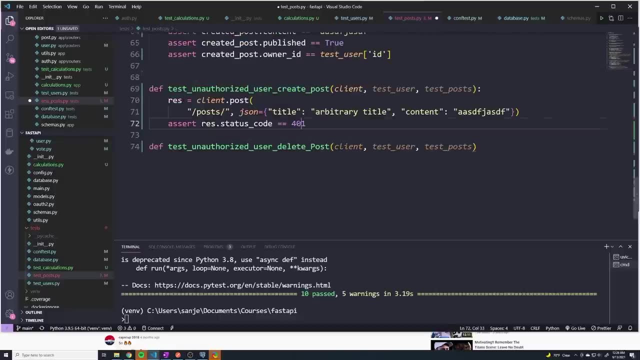 We'll say test unauthorized Oops, Delete Post. And we'll have client test underscore user And we'll definitely need test posts in this case, And then we can essentially copy: well, I'll copy this one right up here And we'll change this to: we don't need the body anymore. 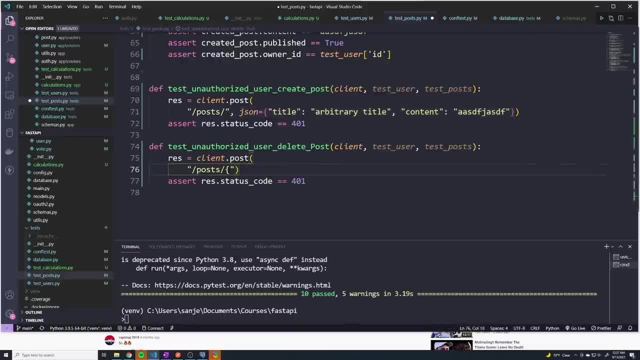 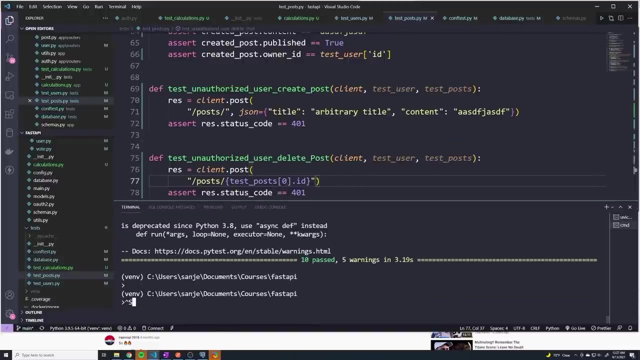 And the route is going to be: We're going to pass test underscore posts, Zero Dot ID. All right, Let's test that out. All right, That's it. test that out. And I realized this should be a delete actually, not a post. That's why 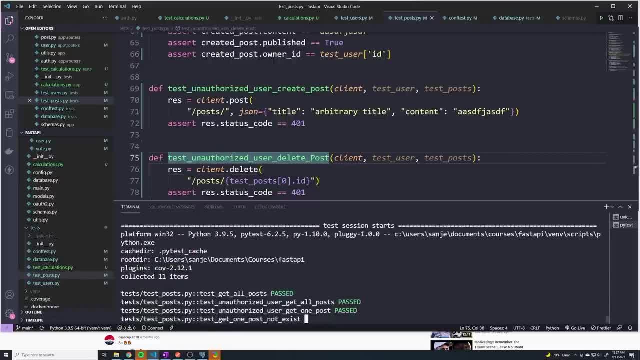 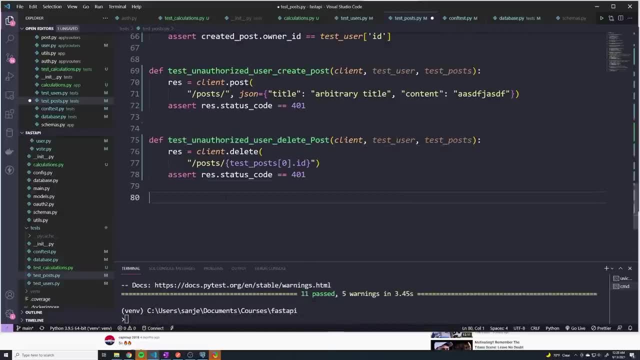 I got some other status code, Perfect Alright, so we got that one to pass. And so now let's test a valid deletion. So I'll say test, delete post, And ideally I guess we should be calling like success, like we successfully deleted it, And this time we'll get the authorized underscore. 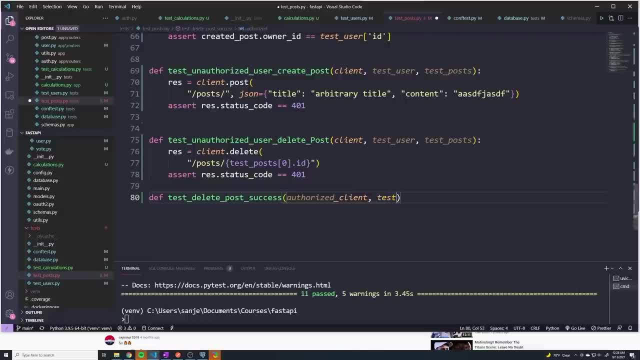 client. We'll get the test user and the test underscore posts. Alright, we'll call this same request here And just change this to authorized client, And this should give us a 204.. I mean, you theoretically could also, you know, then fetch all posts again. just to verify that. 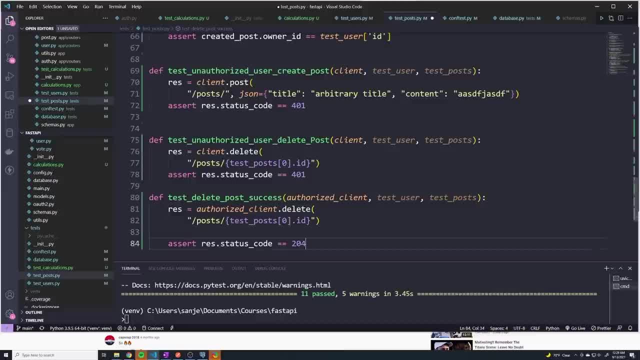 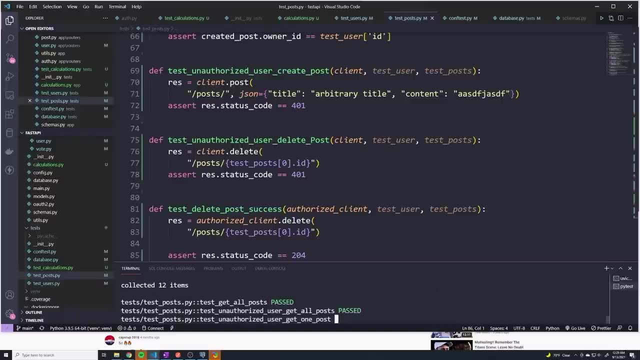 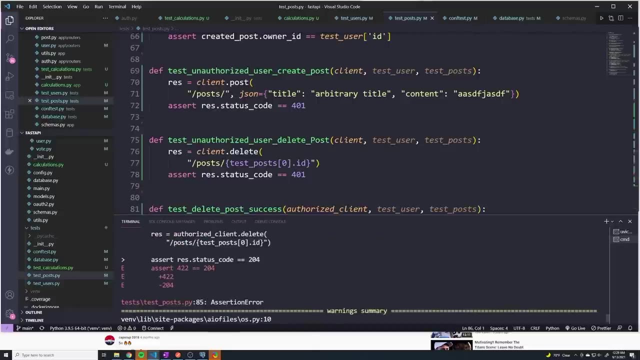 the total number of posts is one less, But we're not going to do that In this case. you could, however, do that, And that failed. So what happened here? a 422.. And two things. So I don't. 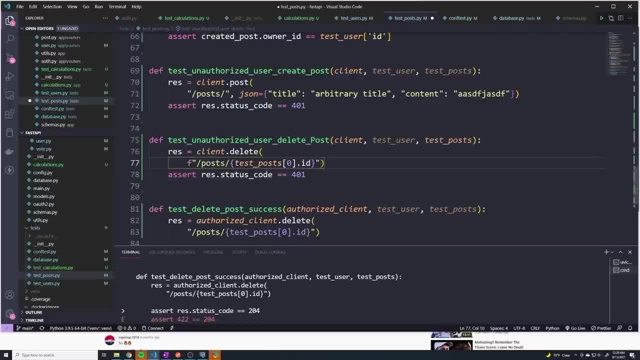 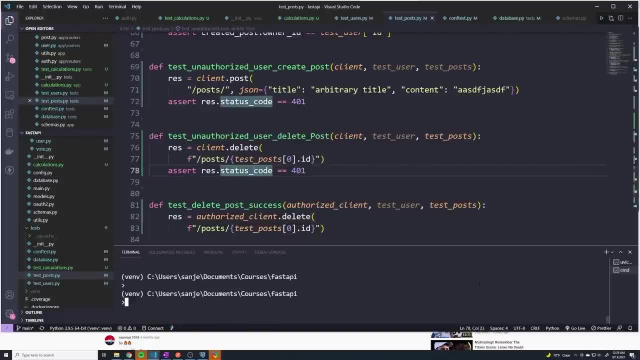 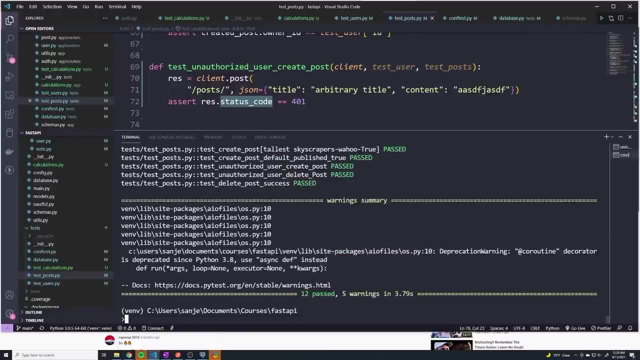 even know how this one ran with the same issue. we should. we need to make that an F string, So I genuinely don't know why that actually worked. Little alarming, but let's test both of those out. Alright, all of them passed. So we've got that. 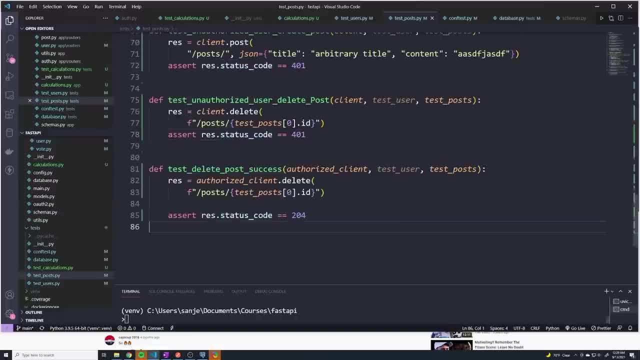 done. Let's test deleting a non existent post, So an ID that doesn't exist in our database. I'll say test delete: post non exist And I'll just copy these And I'll copy this. actually, I'll just copy all of this And 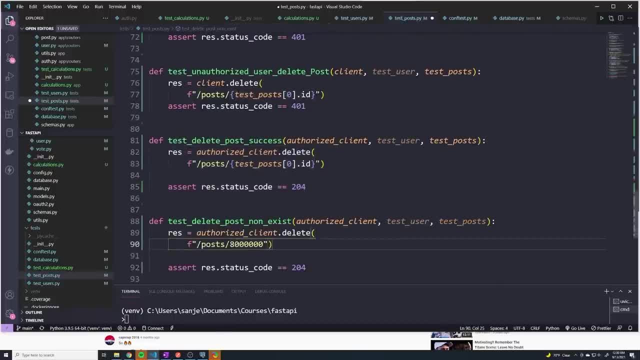 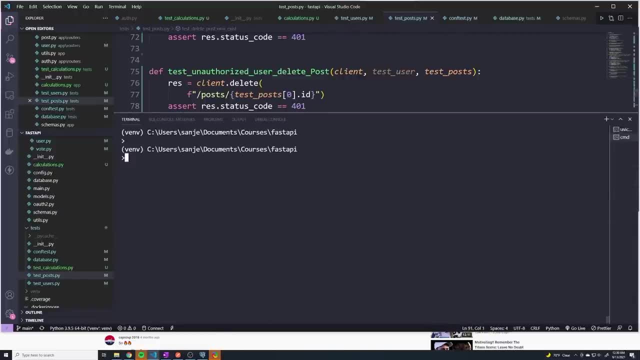 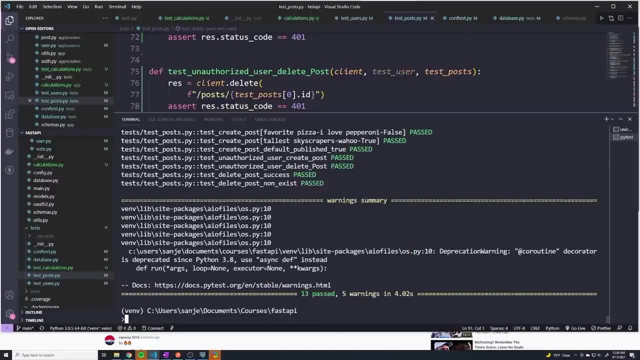 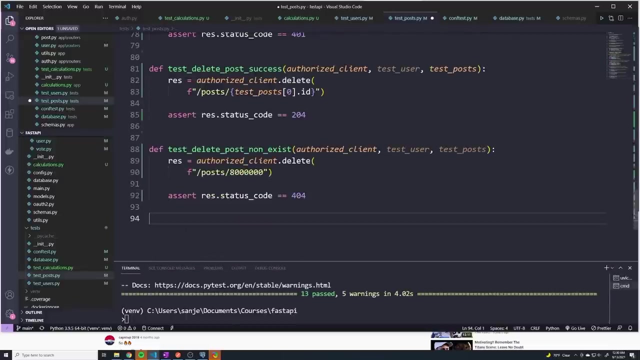 I'll just change this to be some ridiculously high number, And this should be a 404.. Alright, that one looks good. Alright, so the next one is going to be a little bit trickier. We're going to create a test where a user tries to delete a post that isn't theirs. 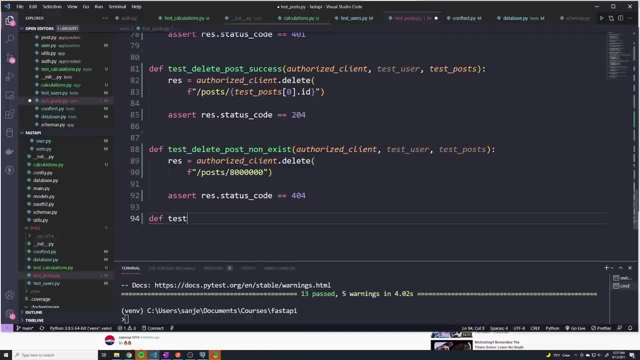 They try to delete a post that's owned by someone else. So we'll say: test, delete other user post. Now there's a couple of issues here. So first of all, we need to actually have more than one user In the database and we need to have posts owned by multiple users now. So this creates 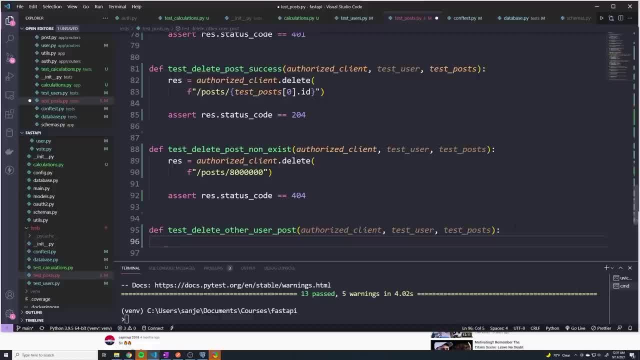 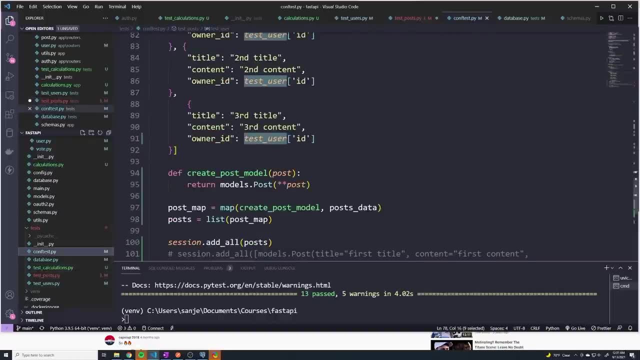 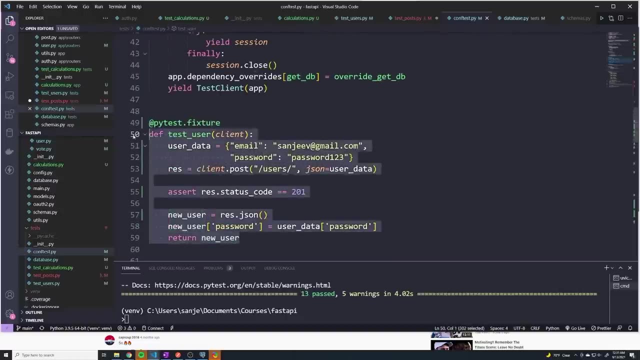 a couple of challenges. So how exactly are we going to set up more than one user? Well, I think it's best to use fixtures, like we always have, And ideally, I would have set up a test user. Where is it, my test user? I would have set up a test user to actually 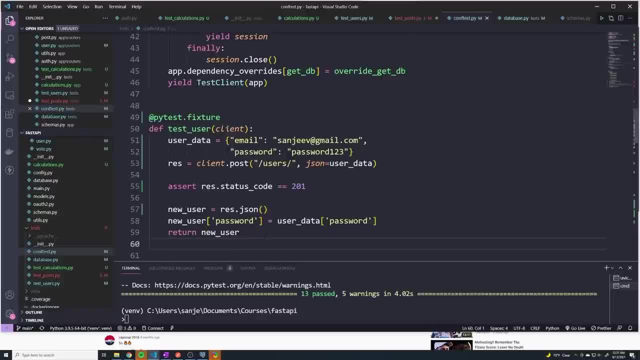 create multiple users in our database, but I didn't, So I just have one. If we had set it up to the multiple user in the database, then this test would be a little bit easier. Since I didn't, what I'm going to do is- I'm essentially going to copy this. I'm going to 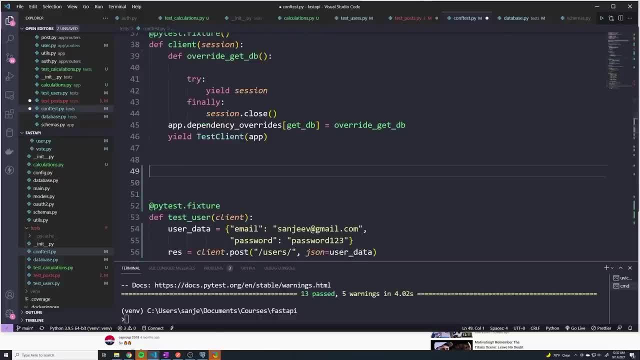 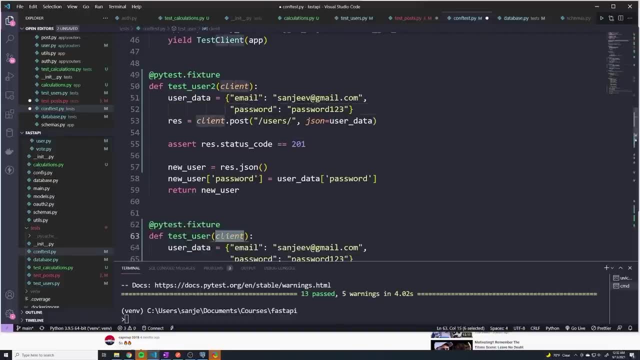 copy this And right above it I'm going to create just a second one. I know it's not very original, probably not the most efficient way of doing things And it's gonna be dependent on client And we're just going to put a one or something- it doesn't really matter- just so that we have 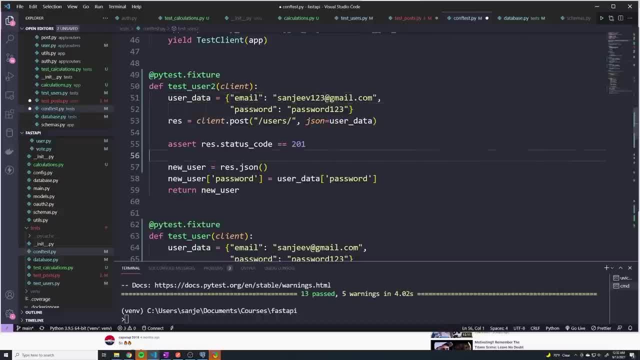 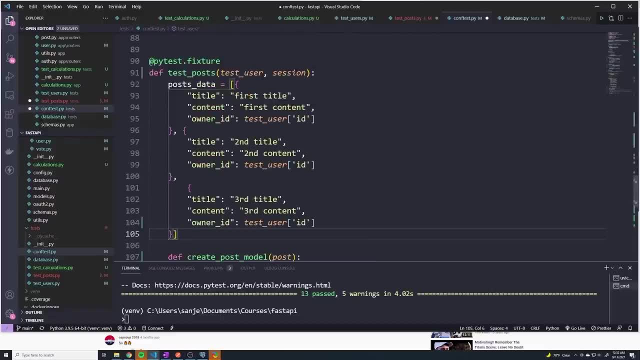 another user, I'll make this 123.. And so now we have two users, Which is perfect, And down here in my posts data. what I'm actually going to do is I'm going to create one extra post And we could just copy this data right here. 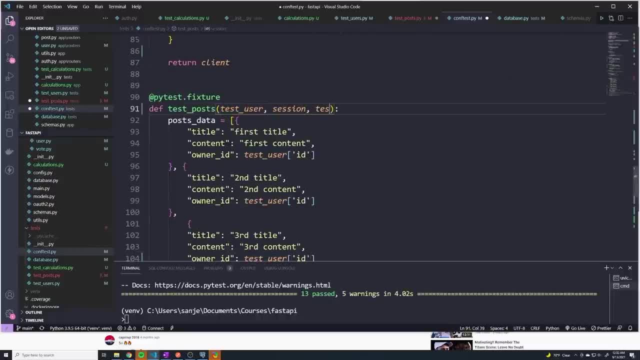 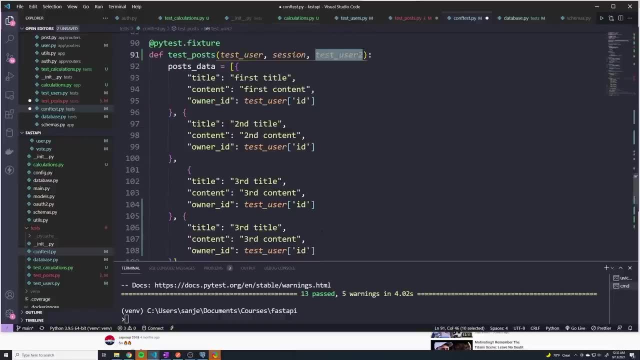 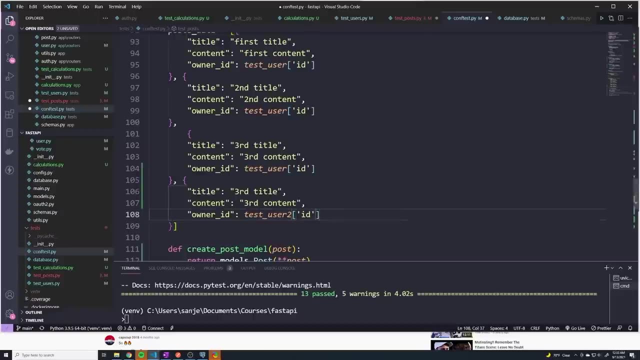 And here I'm actually going to pass in an extra fixture which is going to be test underscore user two. So before test post gets created, we're going to create the second user And here I could just grab the ID of test user two, And actually I don't even need to do that. I don't know why I did that. Let's. 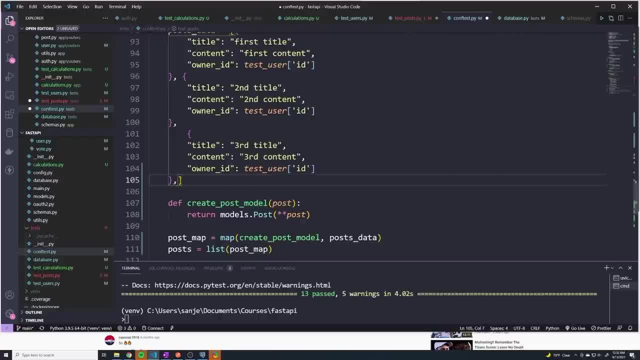 we don't even need to create a post owned by that user. We'll leave it like this for now. Nope, I was right. Actually we do. I don't know why I'm flip flopping like this. So So the fourth. 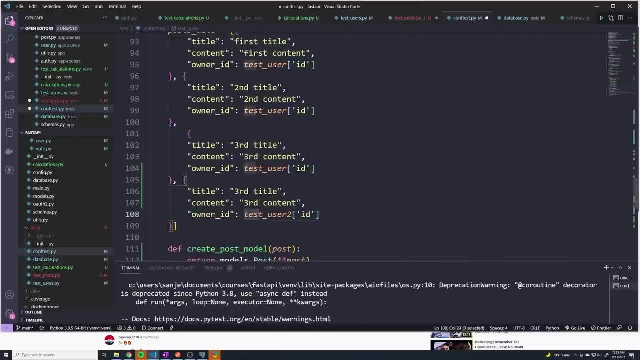 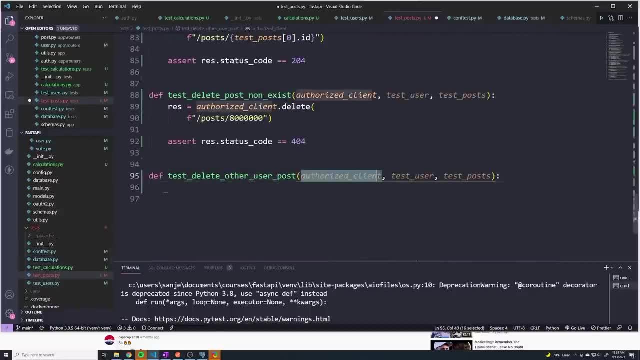 post 1234 is going to be owned by test user two, And so now, if I go back to test posts here, we're going to be logged in. Remember, authorized client is always going to be logged in as user one. So we're going to try to delete that fourth post, And so we can do that by grabbing the ID of the. 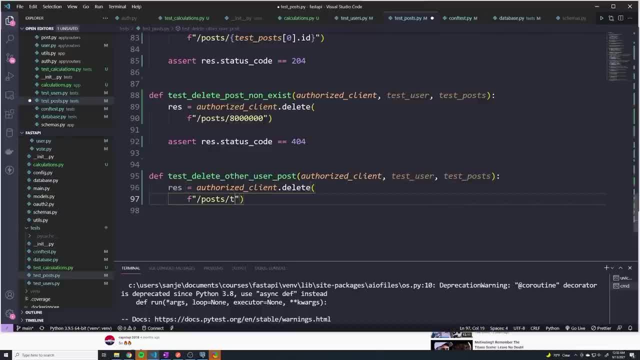 fourth post. So we'll say: test underscore curly braces, test underscore posts. We'll grab the fourth one, which is an index of three, And then we'll grab ID And this, should I forget, what kind of error it should get or what status code. 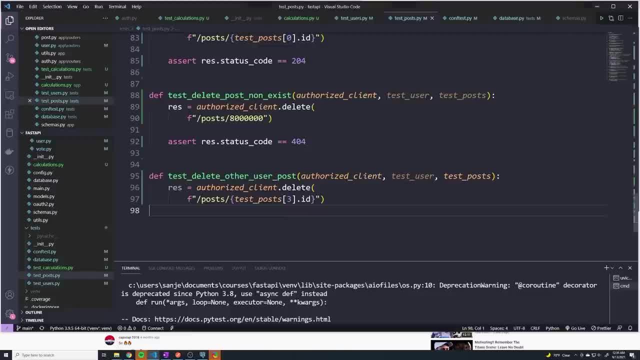 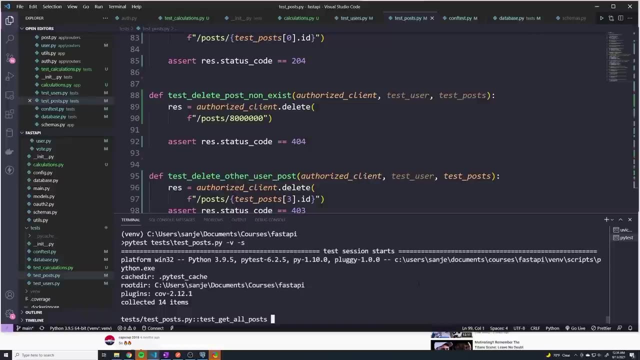 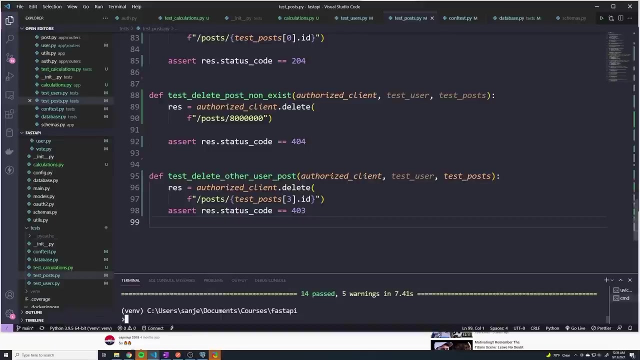 I think it's 403.. So we'll do a cert res dot status underscore code equals equals 403.. And it looks like that successfully passed, And so that one's good, And that pretty much wraps up all of the delete tests that I want. And then in the next video, 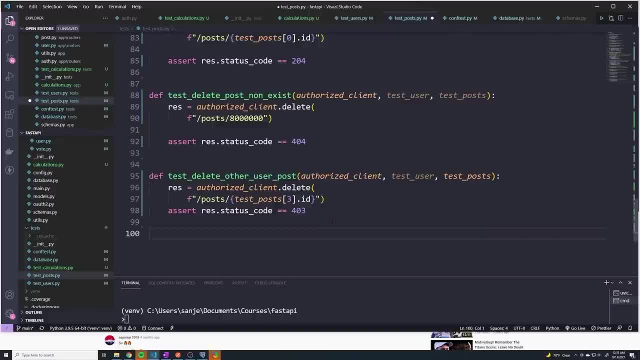 we'll take a look at updating posts. Alright, so let's update a post. also a def, test underscore, update Post. Here we need an authorized client And we'll need a test user And we'll need test underscore posts. All right, and I'm going to define a dictionary, So I'm going to define a. 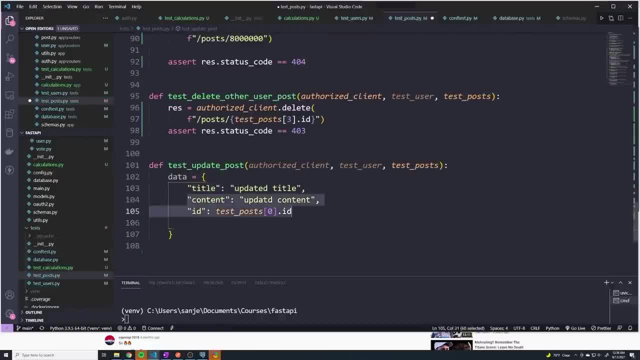 dictionary with the values that I want to update. And so here I've got the title, the content and then the ID which I'm grabbing from test posts, And I'm just going to use the first test post in there And I'll say: res equals authorized client- I think it's put, And then we're going to do an F. 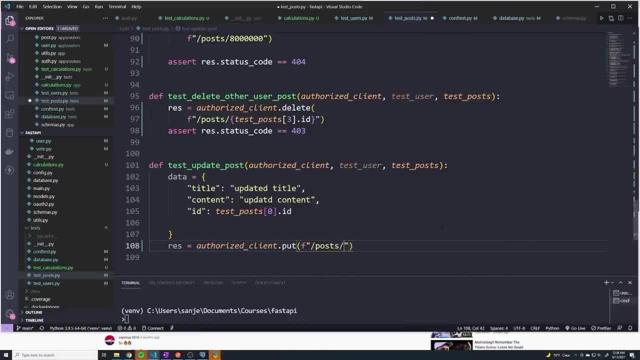 string And we'll say slash posts And this one will be test underscore posts, zeroid. And then we have to pass in the data. So we'll do: JSON equals data. So we're passing in this dictionary Right And, just like we do with the other routes, if we go to the update post. 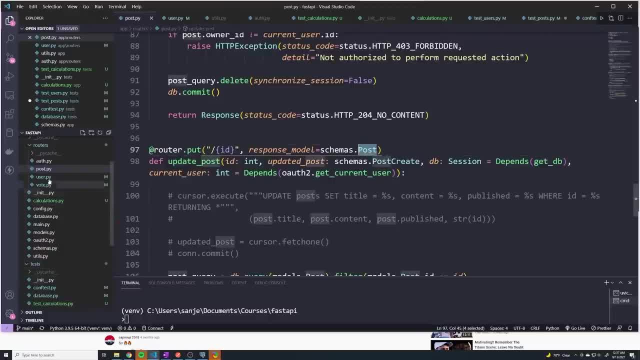 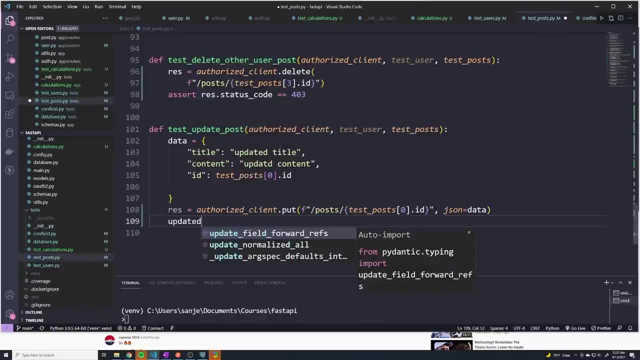 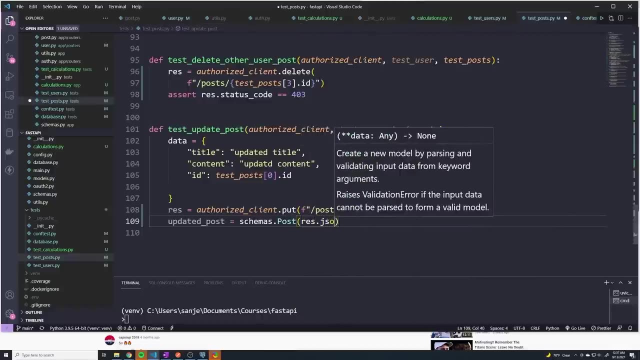 technically we're sending it out with the schema of posts So we can just quickly validate it on our end, on the test as well. So I can say updated post equals schemas dot post And we'll pass in res dot JSON And then we can assert a couple things. So we'll say res dot status code is going to equal. 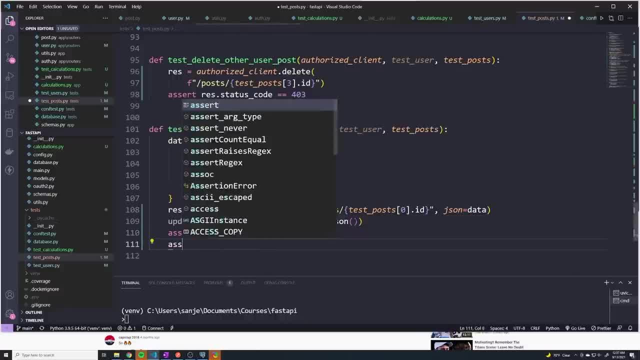 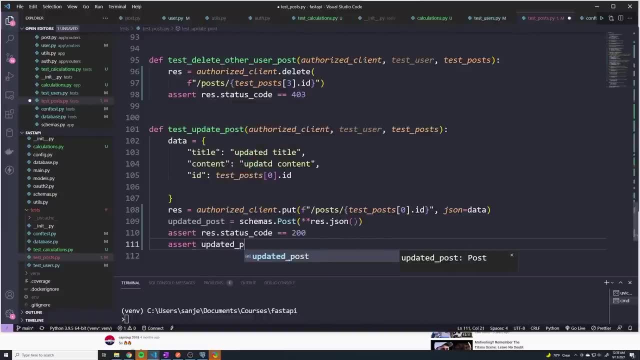 what's an update? I guess we use 200 in that case And then we can assert a few things. So we want to make sure that the new title we can do updated. underscore post dot. title equals equals data dot. updated, Sorry, data dot. This is a dictionary, so title, And we can do the same thing for the. 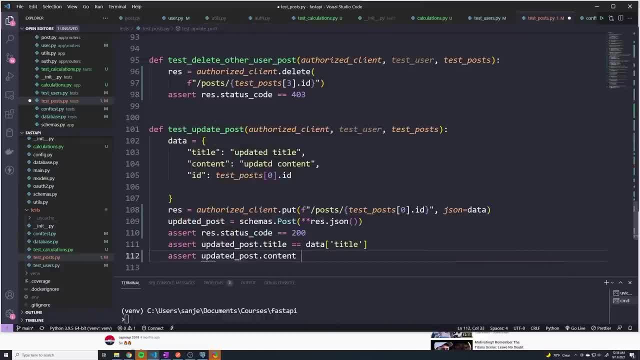 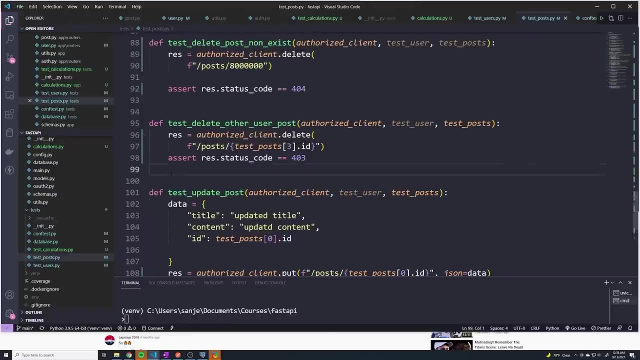 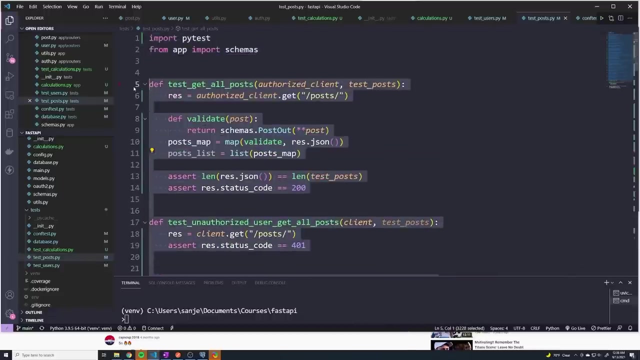 content, And I think that should be everything that we need. And just to you know, just to make sure that my tests don't take too long, I'm going to start commenting out all of my other code, all of my other tests in this file, just to make things a little bit quicker. But you can see how it starts to slow. 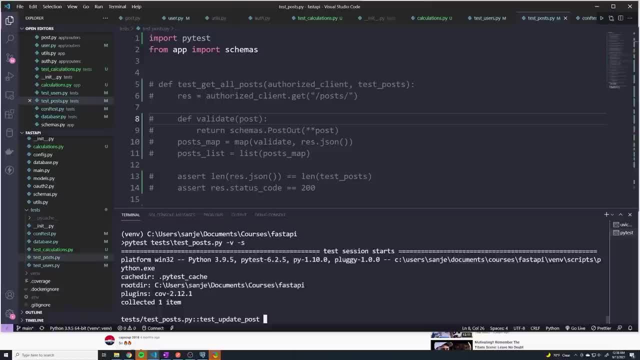 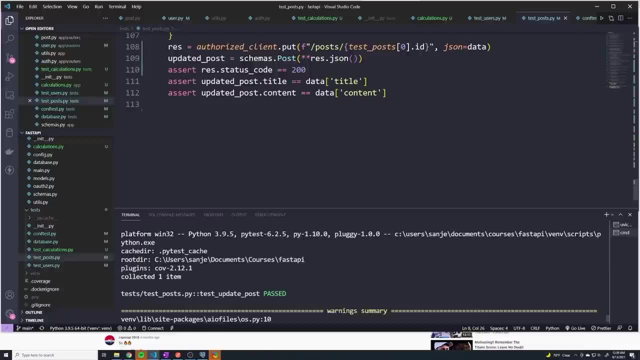 down just with just a couple of tests really, So we can see that it did successfully pass. So that's good, We've got the first update post test. The next thing I want to do is I want to try to update another user's post, So we'll say: update other user. 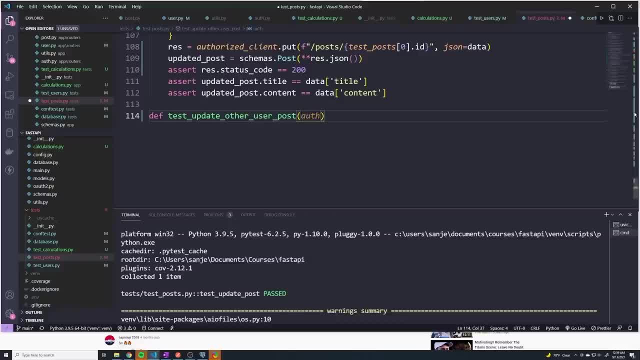 post. So this: we need authorized client, We need test user And we need test user. So we're going to try to update that last post And so I'm going to define a dictionary with the values. I want to update it with So same thing: title content. The only difference is the ID is. 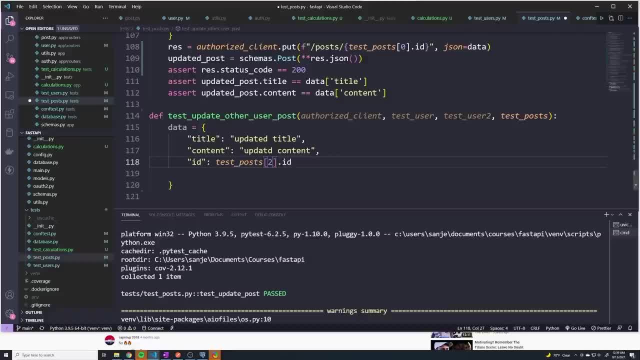 going to be- I think it's actually three. The ID is going to be the third- sorry, the fourth item in that list, And I just want to make sure it's the fourth one. So one, two, three, four, five, six, seven. 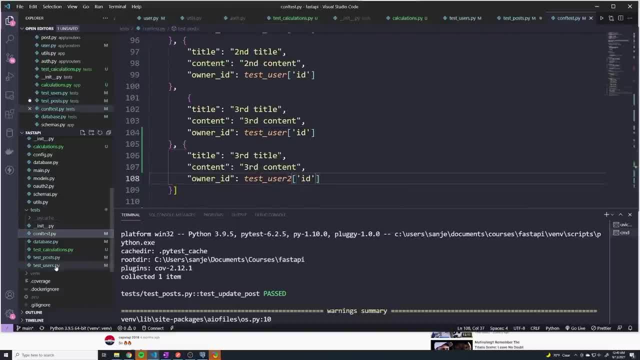 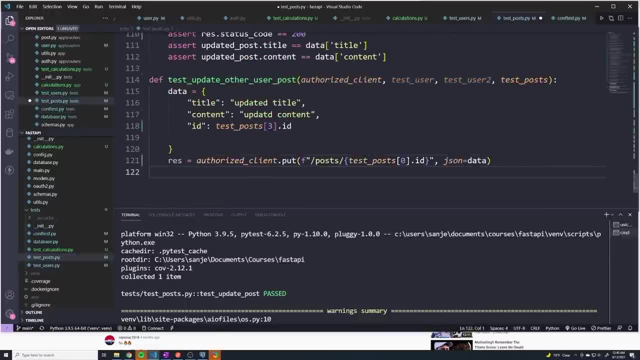 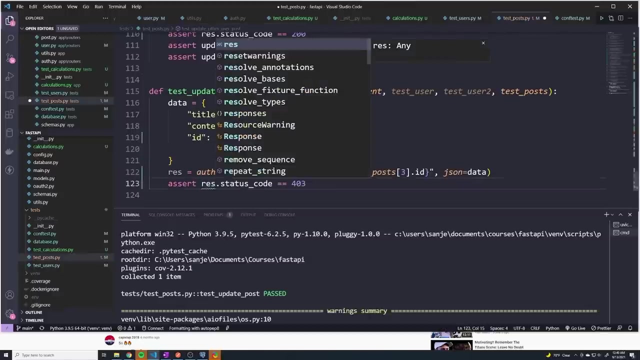 two, three, four. So yeah, we need a value of three, And I'm going to copy this And just change this to three And we should get a status code of 403.. And let's test that out. Perfect, 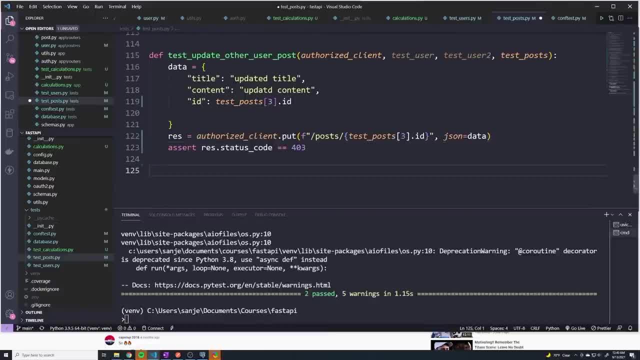 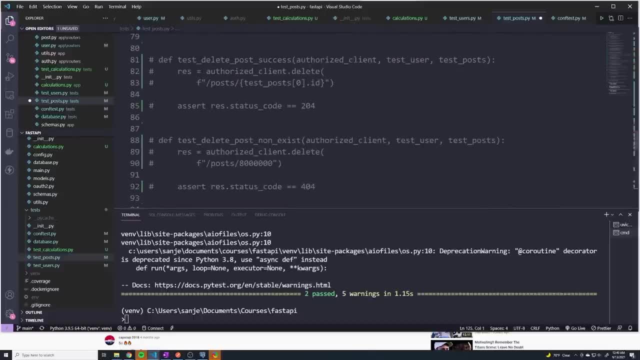 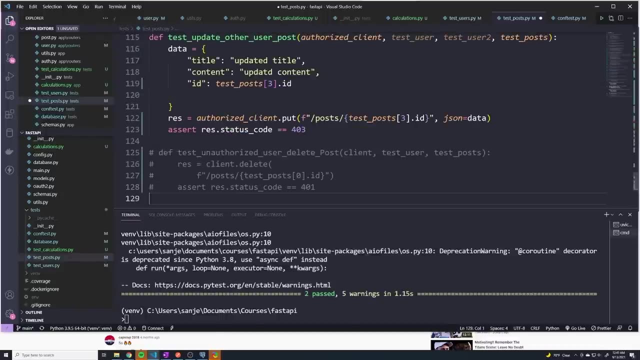 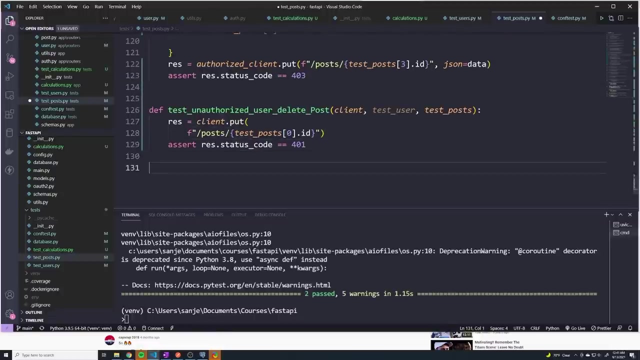 And the last thing we need to do is a unauthenticated user trying to update a post. Actually, there's two more tests, So let me grab unauthorized user, this one right here And this is going to be a put And that should return a 401.. And the last thing that we need is- and actually I need- to update this. 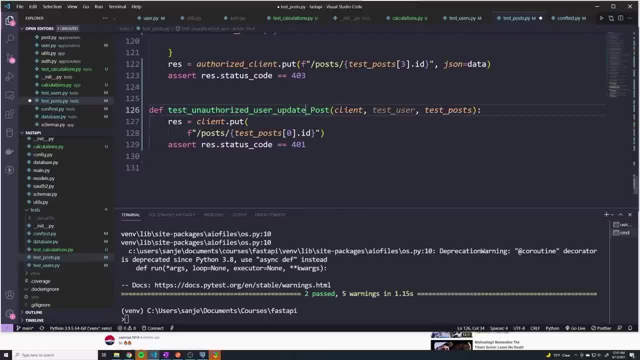 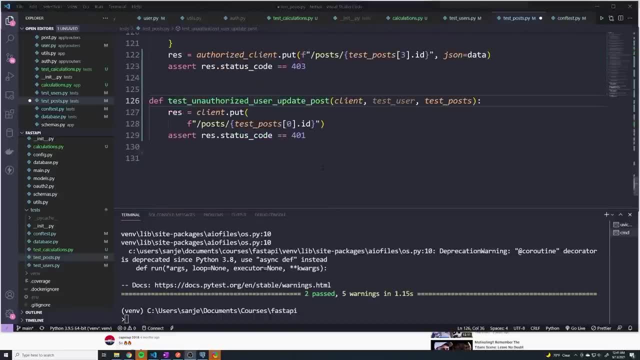 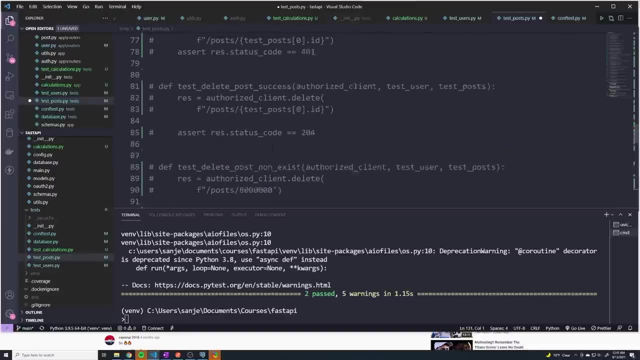 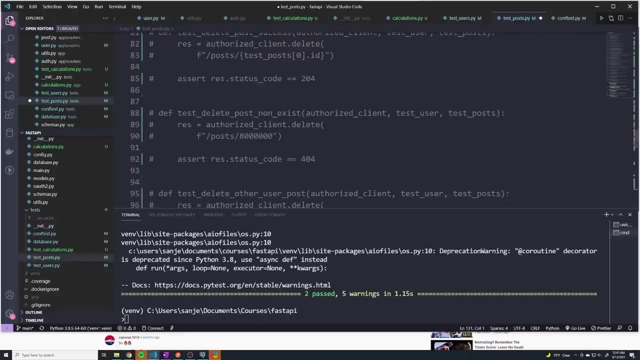 name. So unauthorized test update post. We can also set up a test to update a post that doesn't exist And I believe we can just copy the deleting the post that doesn't exist. Delete post. delete post. non exist, So I can just copy this one. 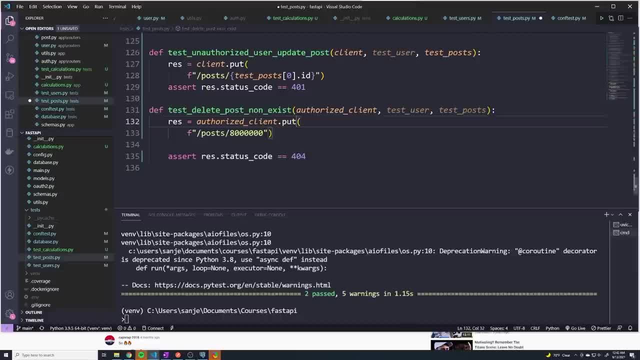 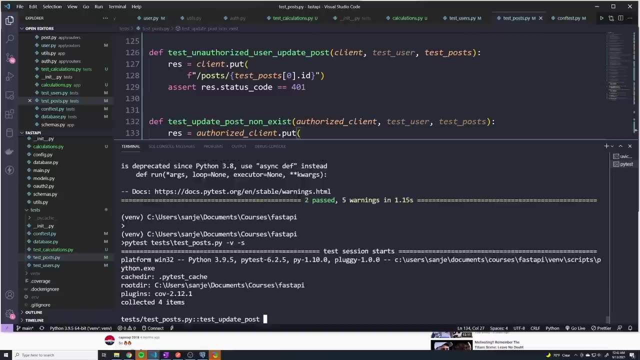 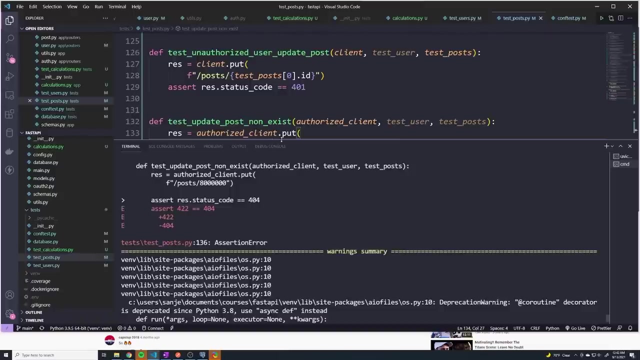 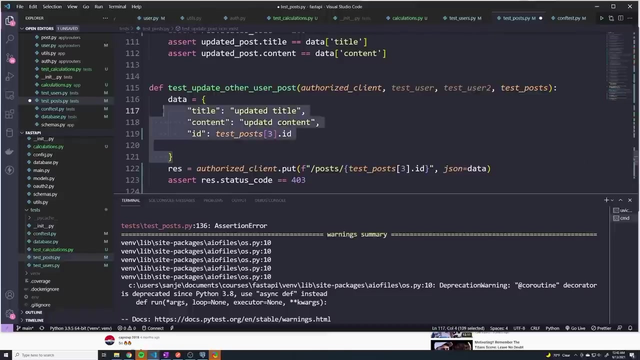 And change this to a put And we'll change the name to be update And let's test this out. Hopefully everything works. Oh, one failed. What happened here? Okay, so it tries to validate it And because I didn't provide any data, so I can just copy this data right here, just so we can give it something. 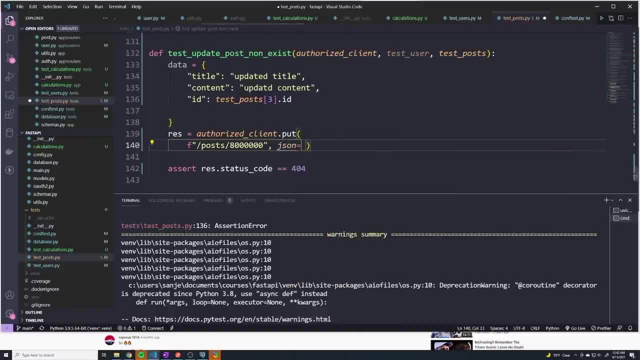 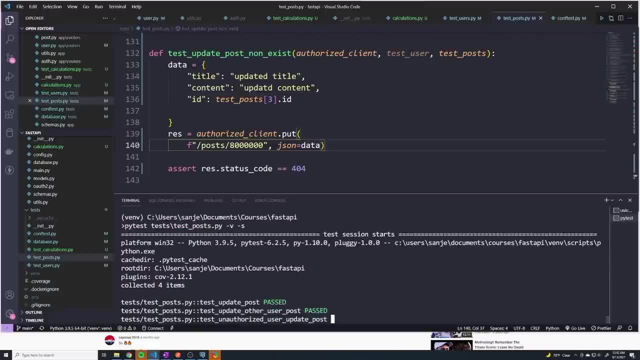 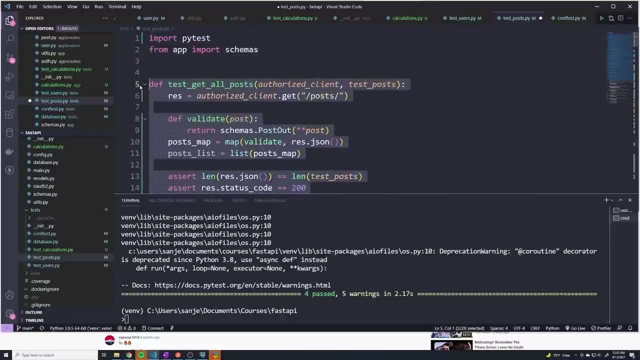 And so we can say: JSON equals data, And that's going to prevent us from getting validation errors And that passed, Perfect. So let's take all that. I'm just going to uncomment everything else so we can get all of our tests back. 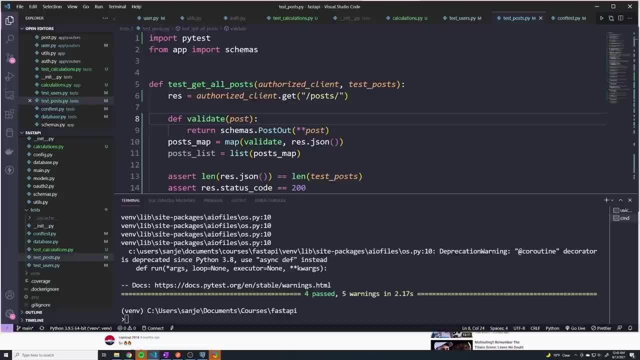 And that's going to wrap up updating posts And that's actually going to wrap up all of my post cases, And so I guess the last thing that we got to do is set up all of the voting tests. Then there's only going to be a couple of voting tests, but it should be fairly quick. 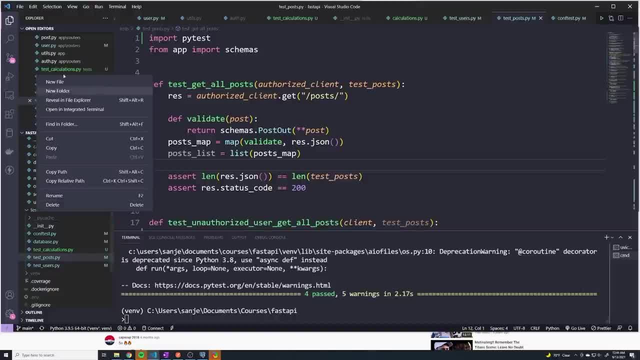 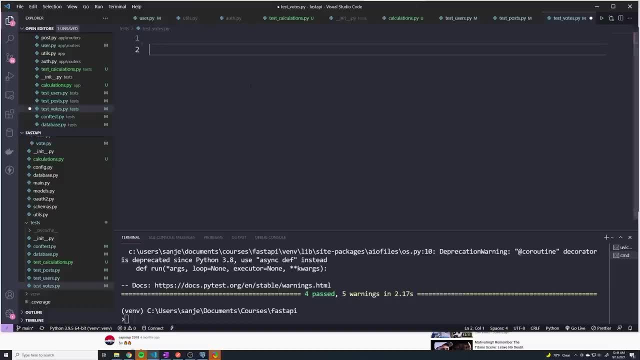 All right, So let's move on to setting up our test for voting. I'm going to create a new file. We'll call this test underscore votes dot py, And let's define our first function. So I'll call this test vote on post. 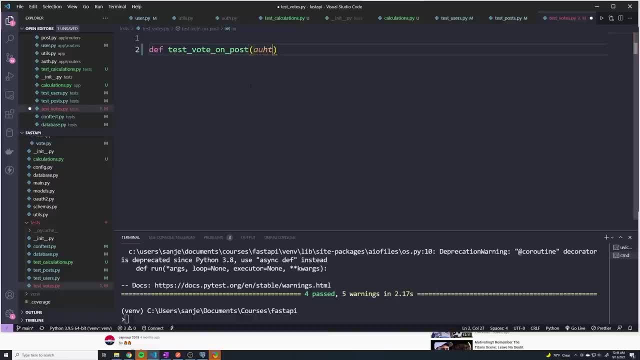 So this is going to be a successful vote on a post. What do we need? We need an authorized client, of course, And we need to make sure that there are some posts already in our database. All right, And now I can do a authorized client dot post. 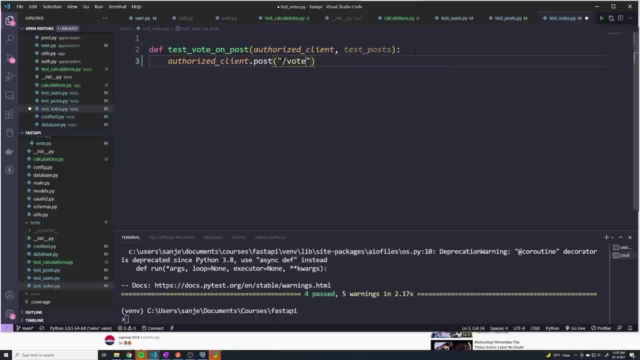 And here this is going to be the vote endpoint And let's just give it some data. So here we're going to pass the post ID, So this will be post underscore ID And we'll grab the first item in our list: Test post dot ID. 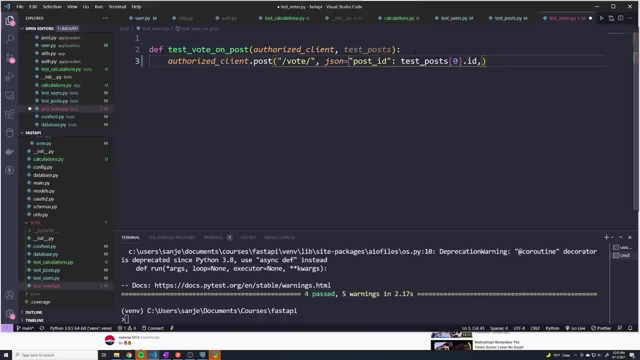 And I forgot my curly braces. That's why it's giving me an error right now And we'll say what is the direction. So we're going to be voting. So this is going to be DuraSet to one, All right. 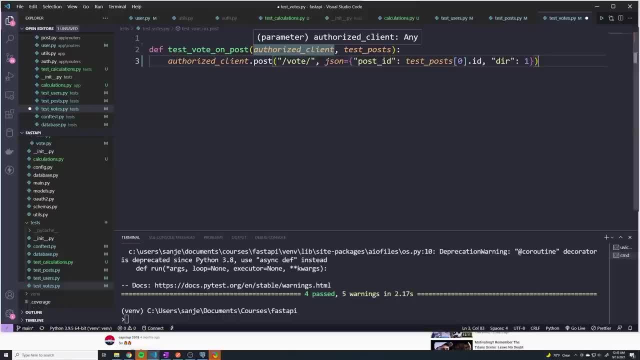 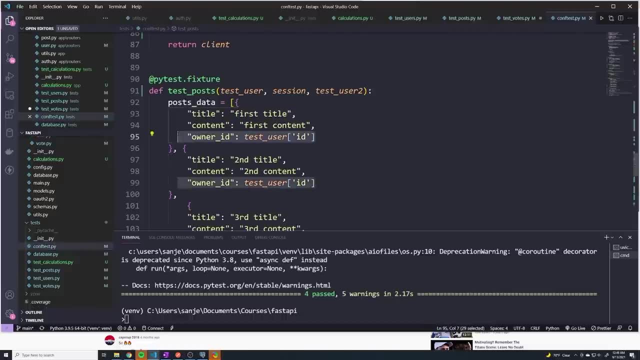 And now, technically, if you look at what's happening right, we're logged in as user one And test post, And if we go back to that fixture, where is this guy? That's owned by user one as well. So technically, we're voting on our own post. 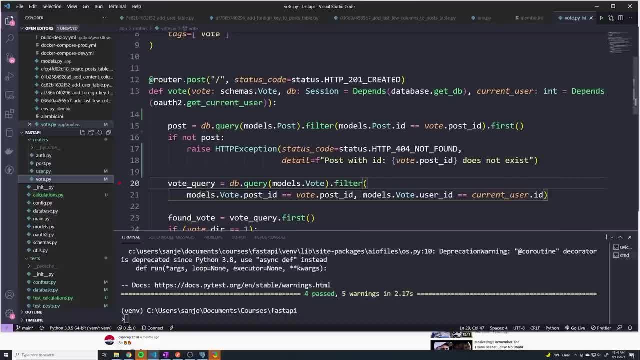 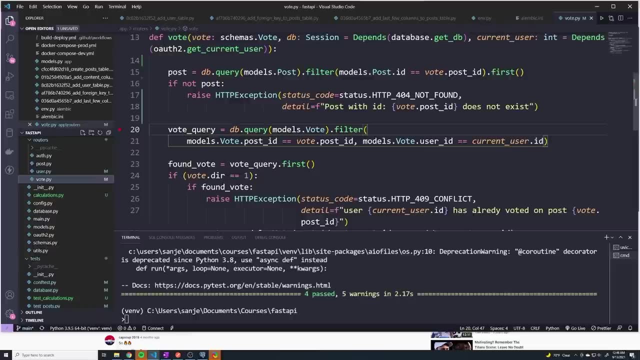 But if you look at our code, we didn't actually put any checks to stop us from liking one of our own posts, So it's perfectly fine in our test to do that, just because our code is right now allowing it. If you didn't want to do it, then first of all we'd have to update this code to make sure that we perform a check to verify that. hey, are we voting on our own code? 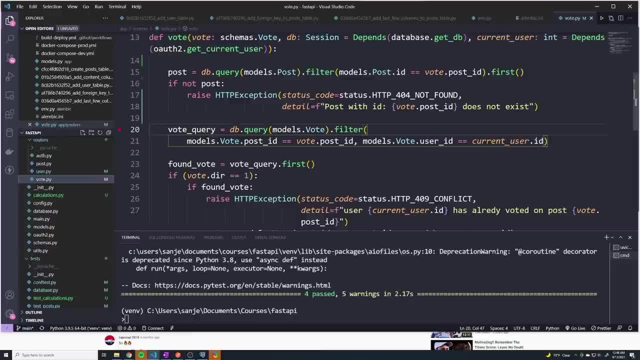 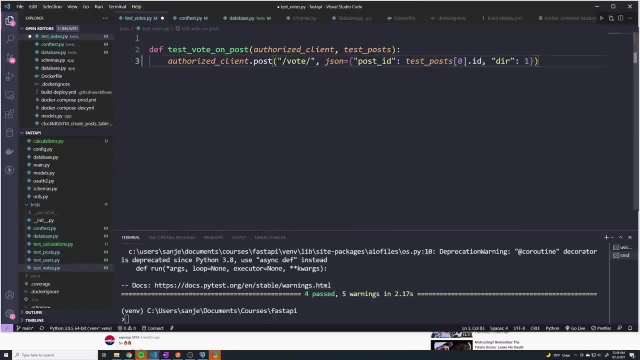 If so, sorry, voting on our own post, then we should reject it. But we don't have that implemented, So for our test, it's perfect. It's perfectly fine because that's how our application works, But obviously, if you wanted to make sure that you're testing someone else's post, then you could just obviously pick the last item. 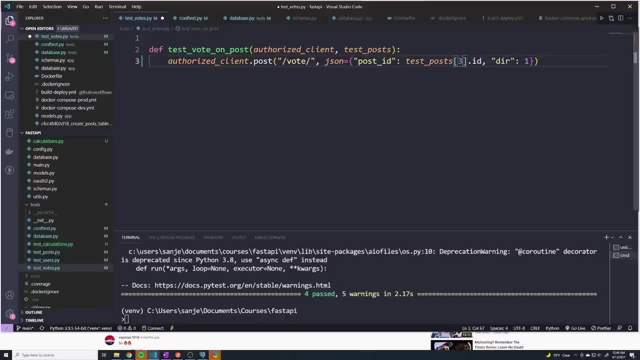 So the third item in the array, because that's owned by test user two- you just would have to make sure that you pass in test user two in this case, Just to make sure that he gets initialized. But that's a good assignment for you guys. 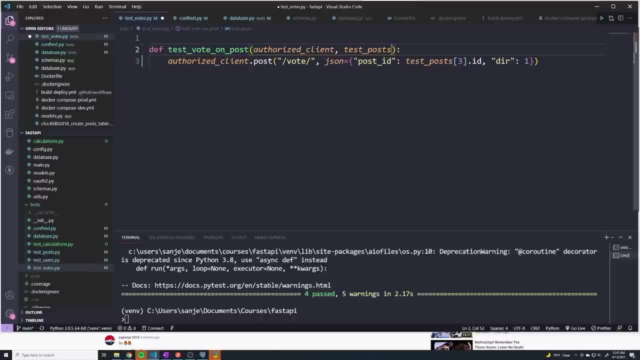 I would see if you guys can implement logic to make sure that you can't vote on your Own post and then go ahead and create your very own test to make sure that if a user tries to vote on his own post, he gets an error of some kind. 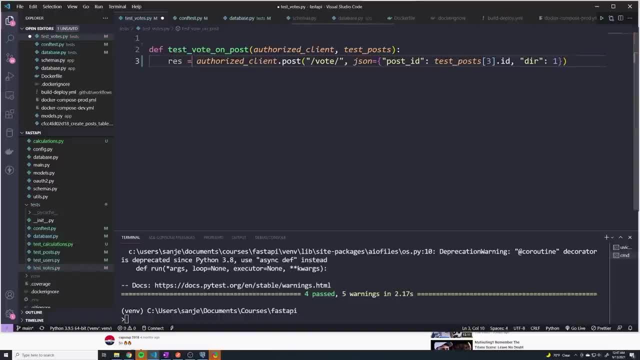 But for us this is good enough. I'll leave it as three, just so we're voting on someone else's post. I'm OK with that, And we can just assert resstatus code: equals equals 201.. Don't really need to check anything else. 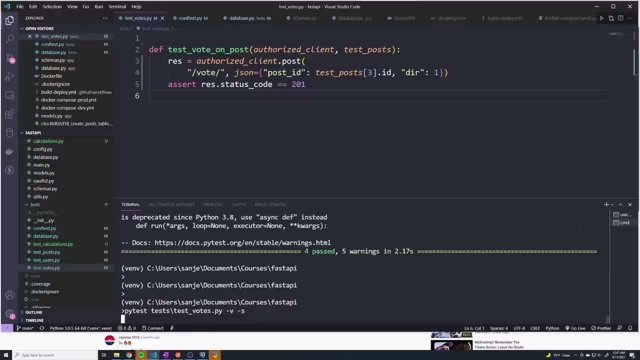 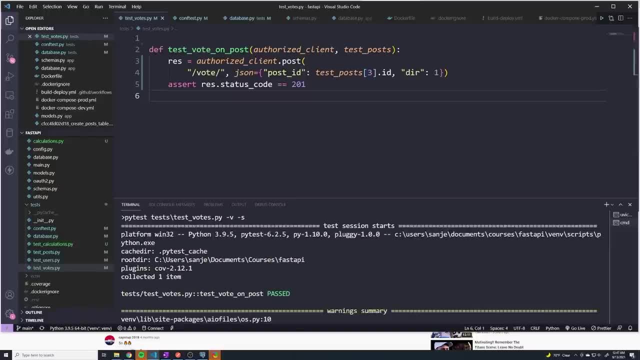 And now I can just change this to test votes. OK, So that one successfully passed, All right. The next thing I want to test on is what happens when a user tries to vote or like a post that he's already liked, So we'll call this a def test. underscore vote. underscore twice underscore post. 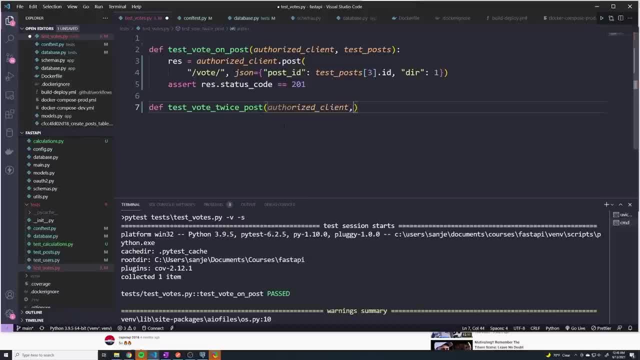 And so we'll need an authorized client. We'll definitely need test posts, But there's one little issue with this one. Right, We need to have a post that's already been voted on, and we don't have that right now, so how do we do that? 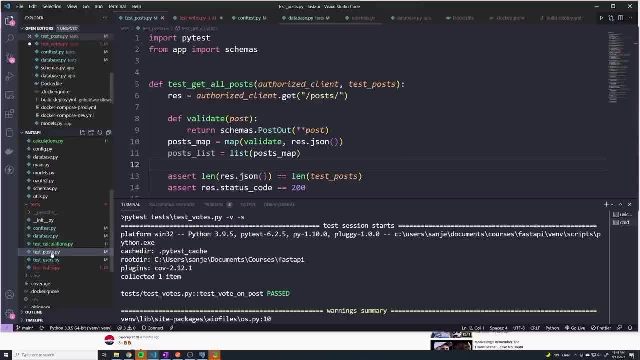 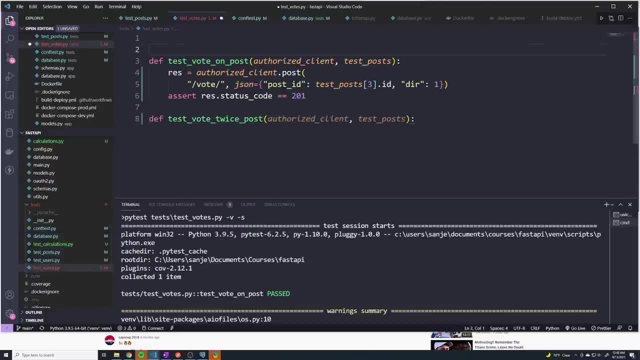 well, i mean theoretically, we could initialize our test post fixture with some votes. but instead of doing that, i'm going to actually create a new fixture and i'm going to keep it in this file, because all this fixture will do is it will set up one of our posts to have a vote on it already. 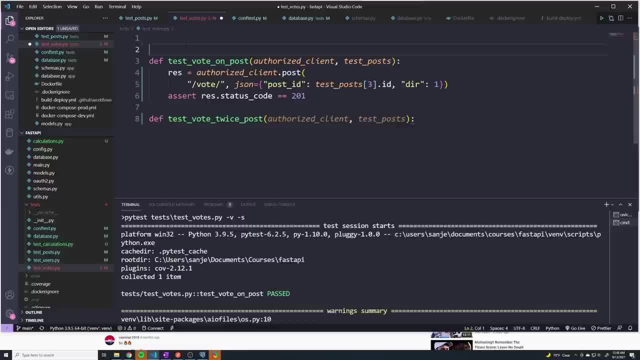 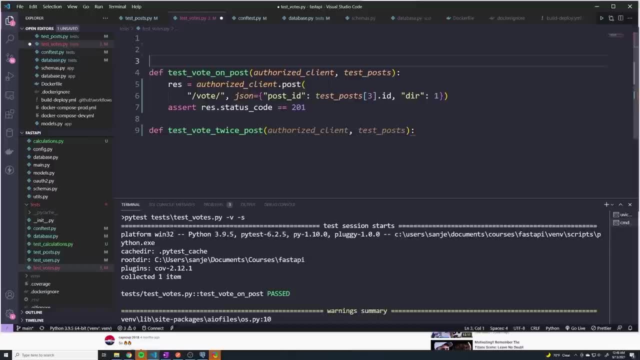 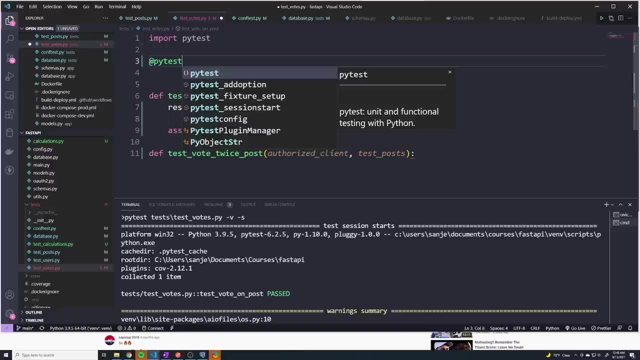 and i don't think really anybody else in any other test in our application is going to need that outside of the voting file, because that's the only one that's concerned with voting. so let's test that out. so we'll import pytest and we'll set up our fixture. so pytest dot fixture. 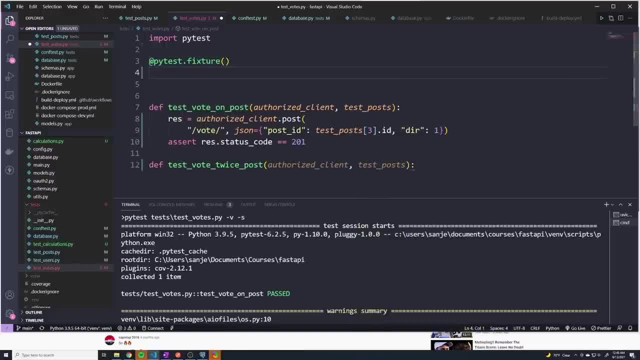 and i'll call this um, test vote, maybe, and and and so for this fixture to work, we definitely need an authorized client. actually, we don't need an authorized client- uh, we'll need a. we'll need test posts: uh, we'll need a session, because we're going to just 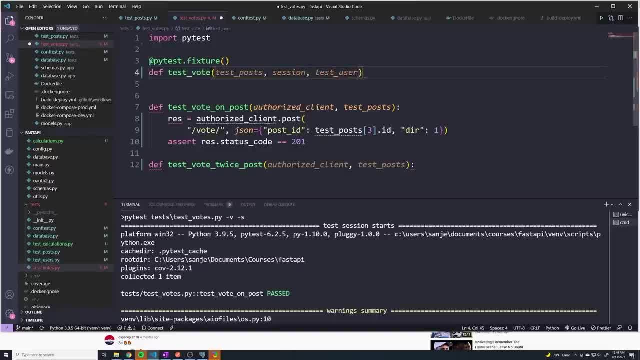 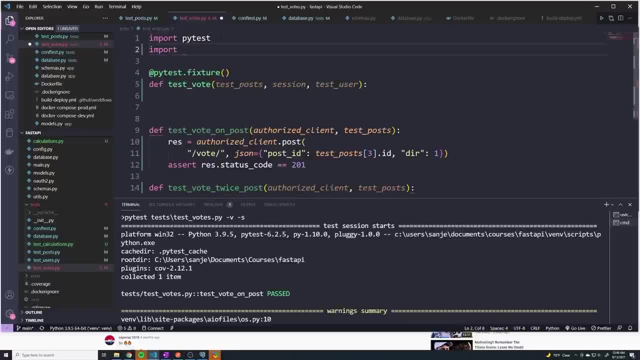 change it in the database directly, and then we'll need our test user and so let's uh. well, we're going to have to import our model, so i'm going to say import uh and import from from from app import models, and i'm going to say models dot vote. so let's create a new vote. 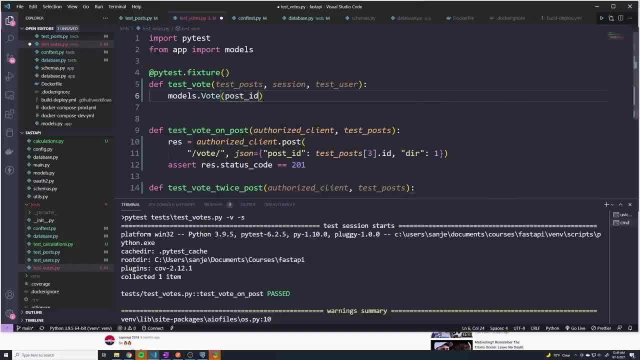 uh, so we're going to have to pass in the post underscore id, which is going to equal test underscore user. we'll grab the third one, dot id, and then we need to pass in the user id, which equals. oh, it looks like we actually. yeah, we already have the test user, so i can say: 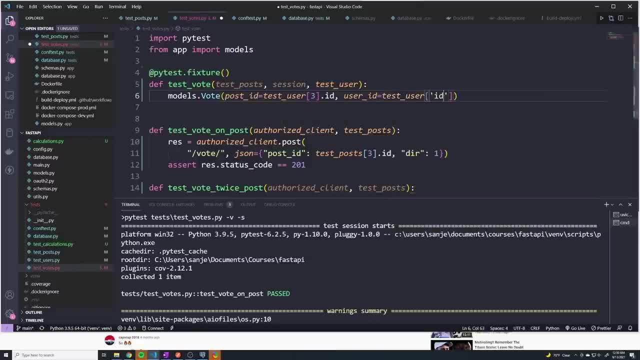 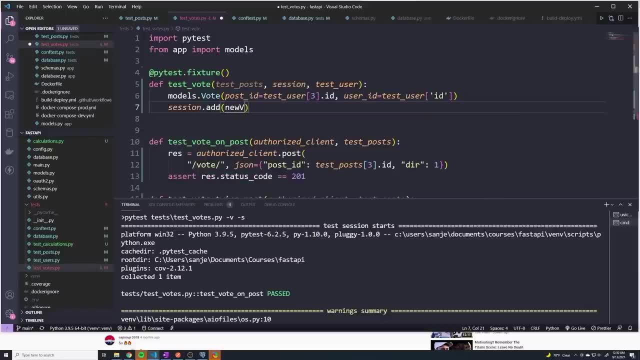 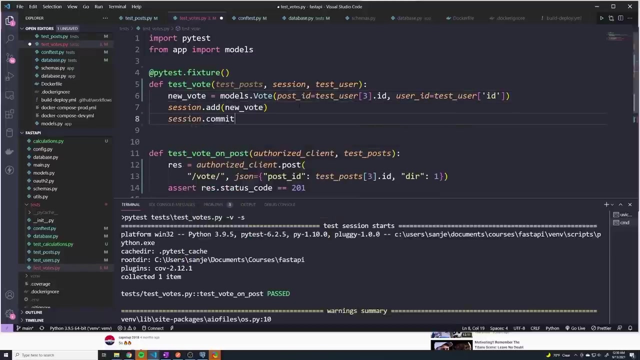 test user underscore user id. and then i can just do session dot, add new vote, and i need to create a variable or store this in a variable. so new vote, and then we can do session dot commit, and so down here i can pass in uh test underscore vote. 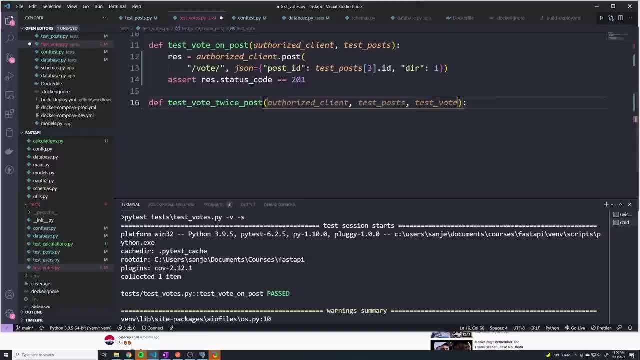 and i'll say: res equals authorized client dot post, and then json equals what is the post id. we'll grab this from uh test underscore posts. grab the third and we'll grab the id and then we'll set the the dir to be a one. so we're trying to revote on that vote. 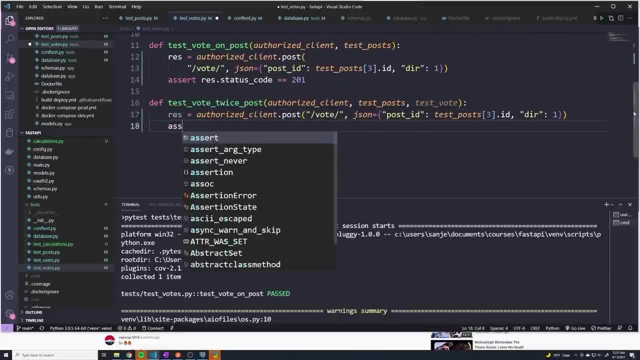 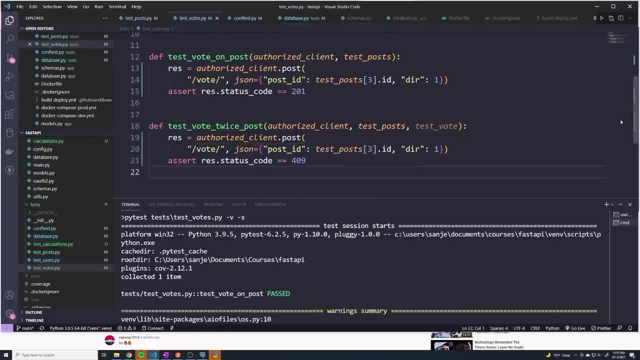 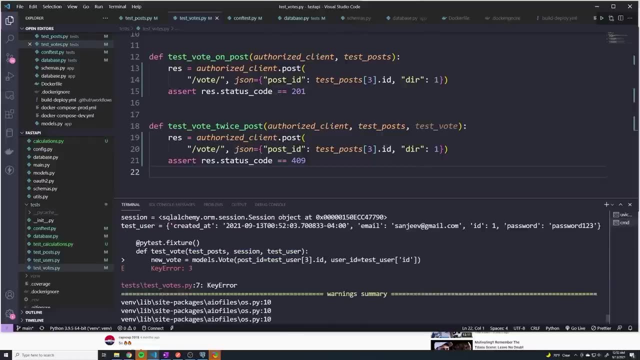 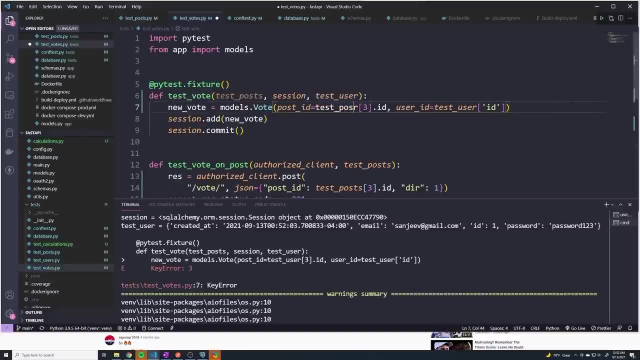 and we should get a 409. so we'll do. assert res dot status code equals, equals 409. all right, let's test that out. one error, oh man, what happened here? that's a key error. so something very simple happened and i see my mistake. this should be test posts. 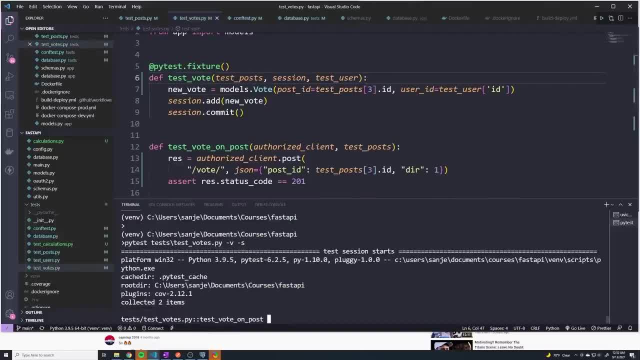 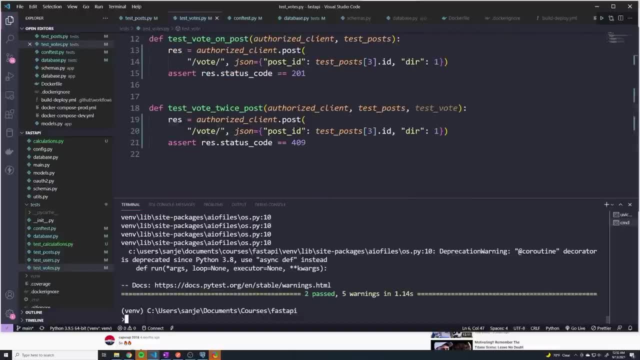 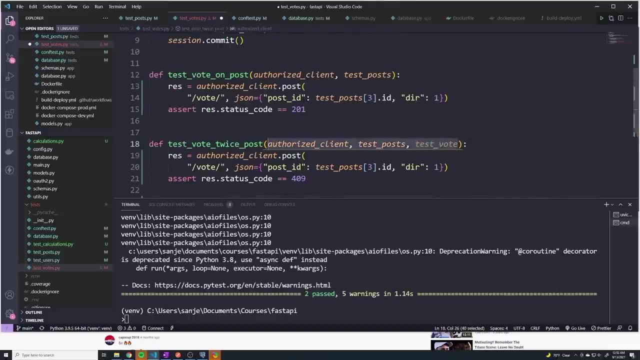 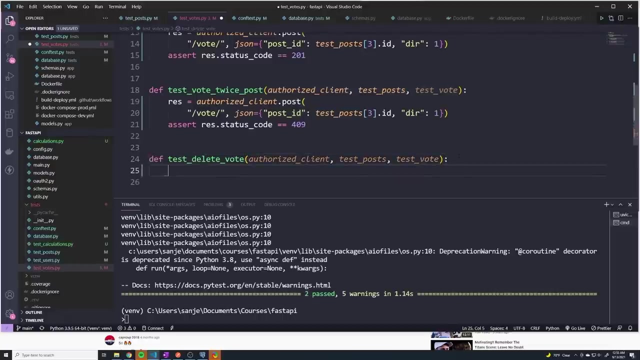 all right, let's try that out now. and that worked, perfect. all right, now let's try successfully deleting a vote, and so we will need all of these. we'll also need a test vote, and so we do. res equals authorized client dot post once again. ugh, i'm just going to copy all of this. 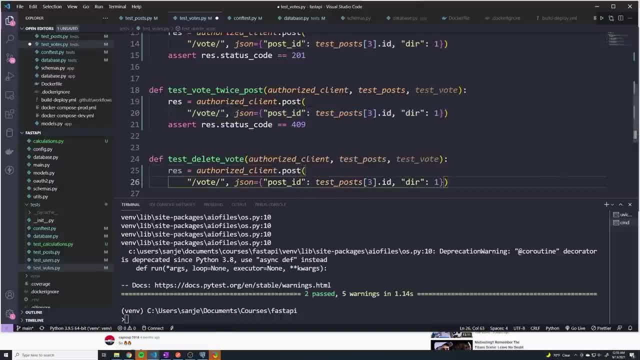 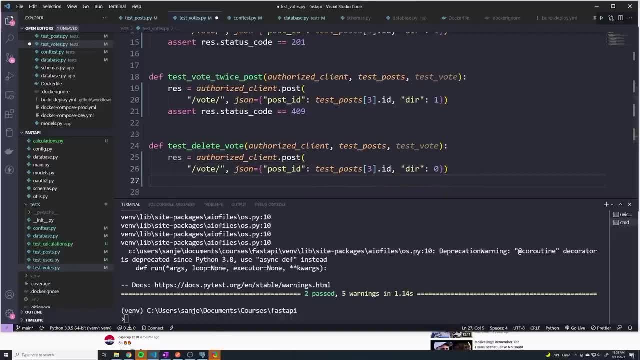 uh, so we got that, and then the direction is going to be zero for deletion, and then we just need to assert res dot status code. uh, this is going to equal. i think we just left it as a 201. uh, this is going to equal. i think we just left it as a 201. 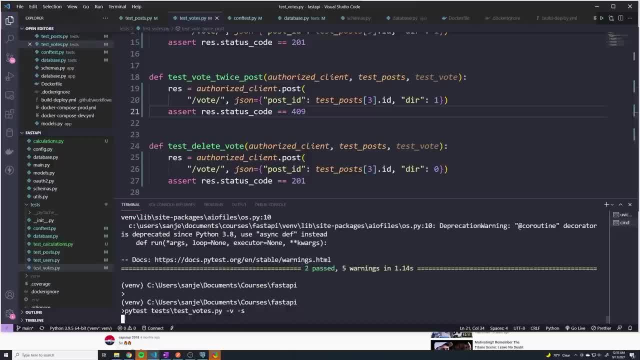 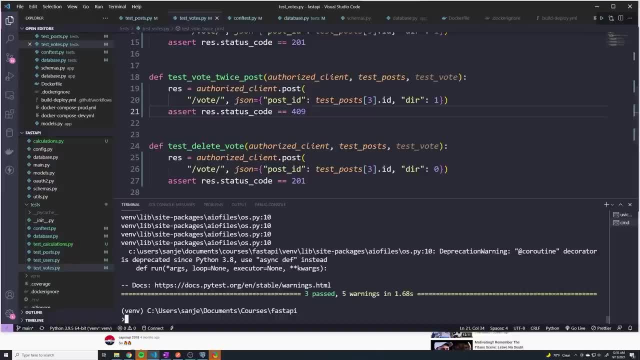 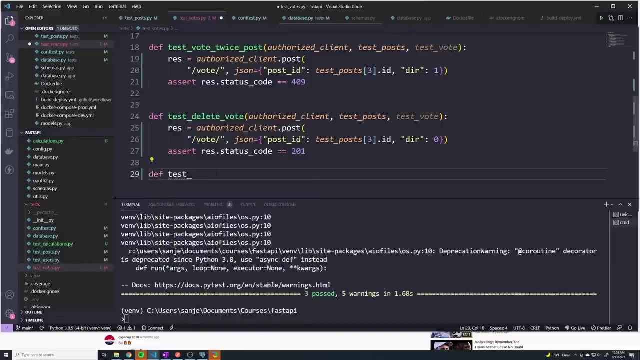 uh, this is going to equal. i think we just left it as a 201, okay, so that worked. and then now we want to delete a vote. uh, that doesn't exist, so, unlike a post, that doesn't that we never liked. so we'll say, uh, def. test underscore. 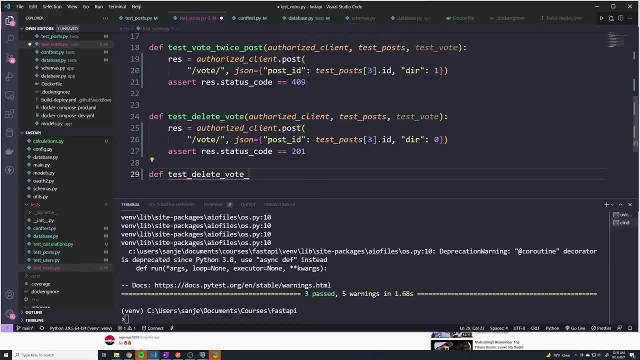 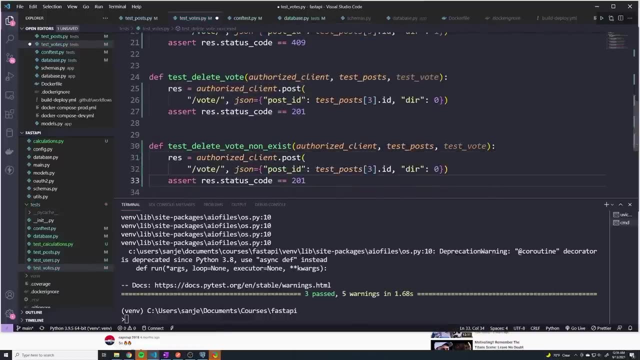 uh, delete vote. none exist, so we'll need the same exact stuff right here. okay, i'm just going to copy all of this for now and then we'll change up the few details. uh, direction zero: same post, um, but i'll just grab. actually, um, we don't want the test vote. 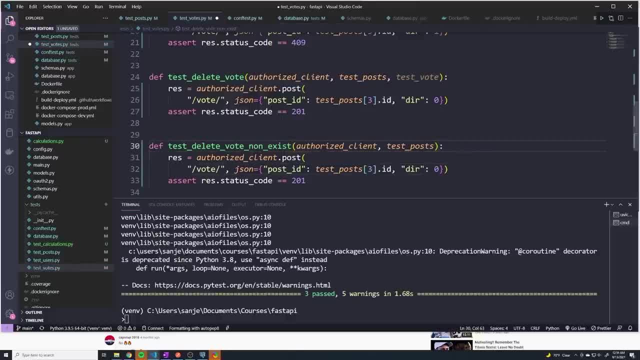 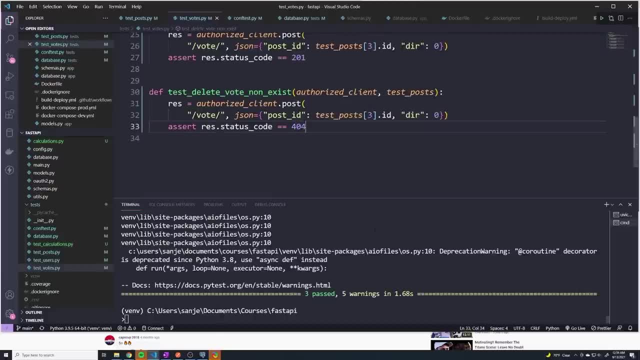 because we want to make sure that there isn't a vote. so we're going to remove that fixture and this should be a 404. let's try that that worked. and then, finally, let's try- uh, voting on a post that doesn't exist. so we'll say: 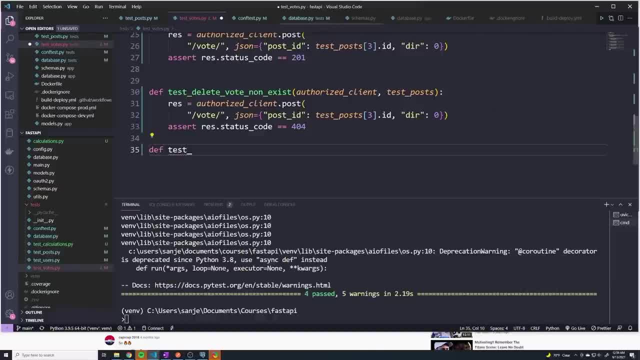 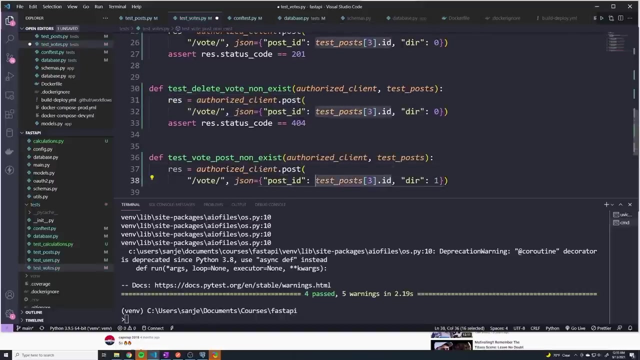 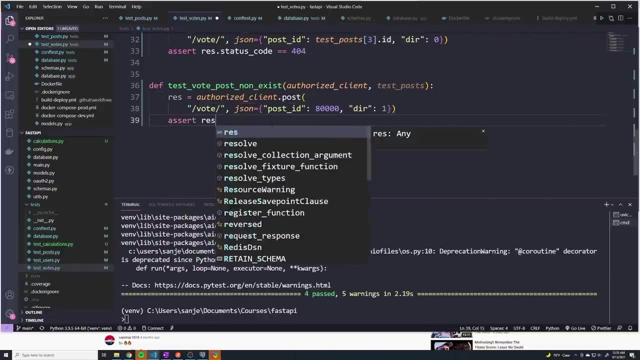 yeah, liking a post that doesn't exist, so we'll say def toast. uh, test vote, post none exist, and uh copy all of these. i copy this, set the direction to one and uh, the id is going to be 8000 and we expect the status code to be: 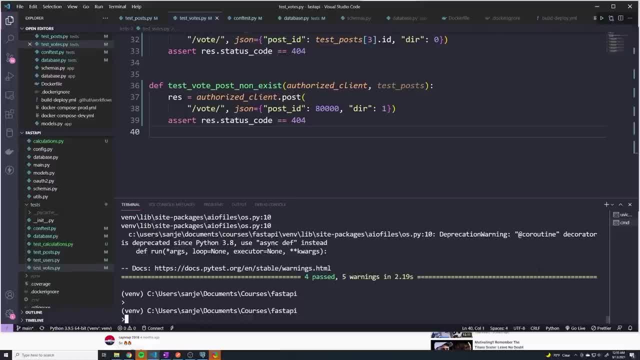 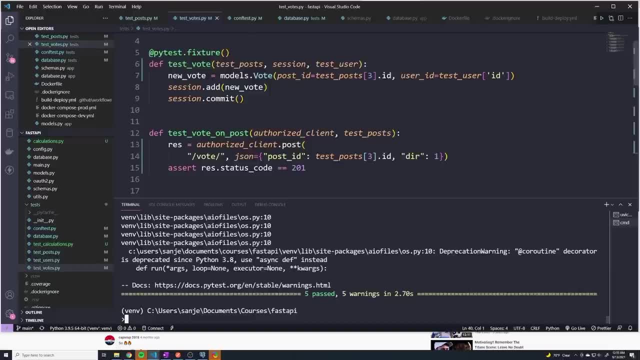 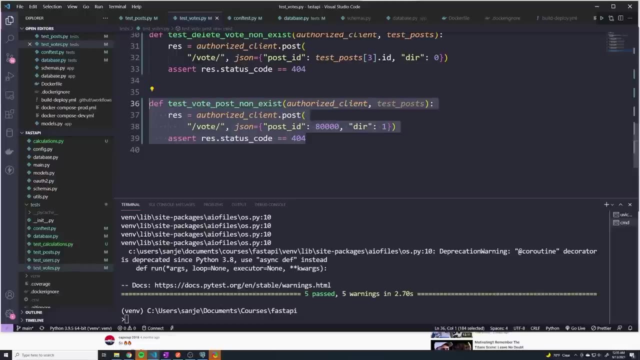 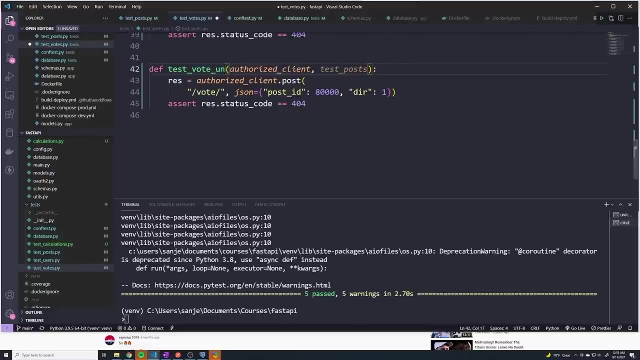 404 as well. all right, it looks like everything's good. the last thing that we just want to check is make sure that a user who isn't authenticated can't vote. so i will copy this: uh, test vote um unauthorized user, and then we want just the regular client, in this case. 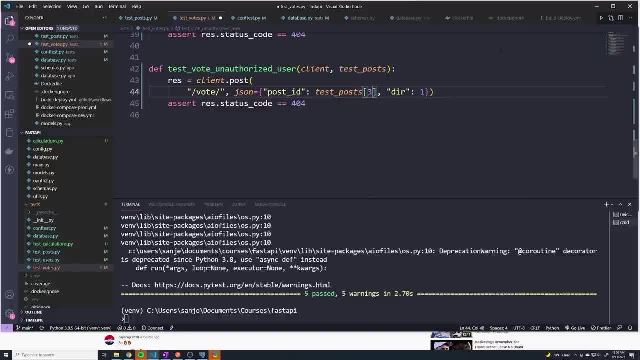 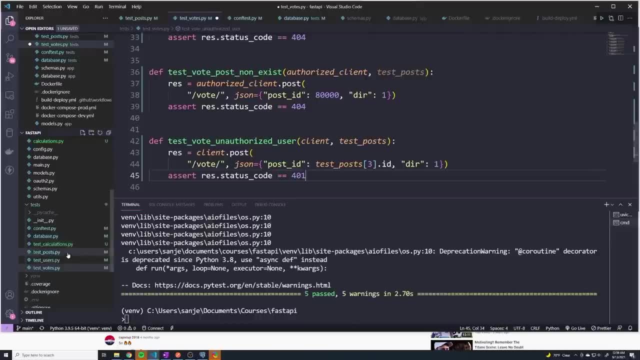 we'll do uh test posts, three dot id, and this should be what? is it a 401? um, i can't remember. let me go to the other one. it should be a 401. okay, all right, guys. so i think we've covered, uh, all of the tests that i wanted to cover. 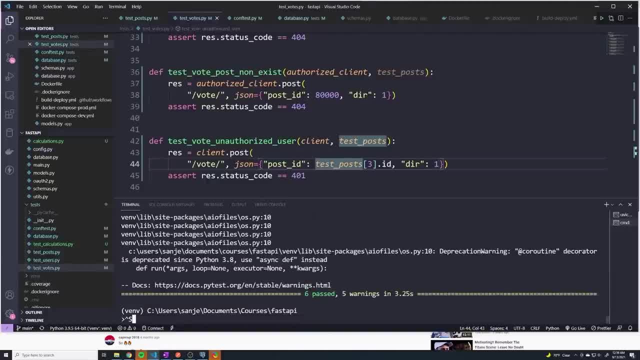 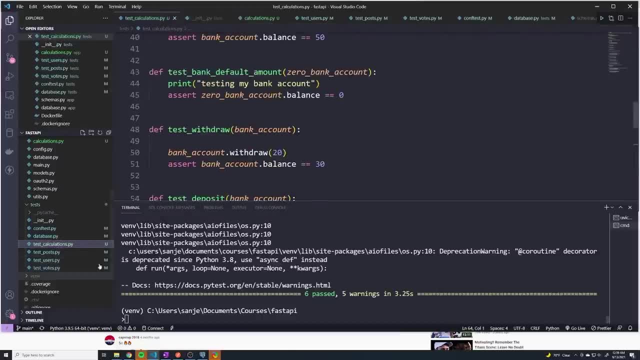 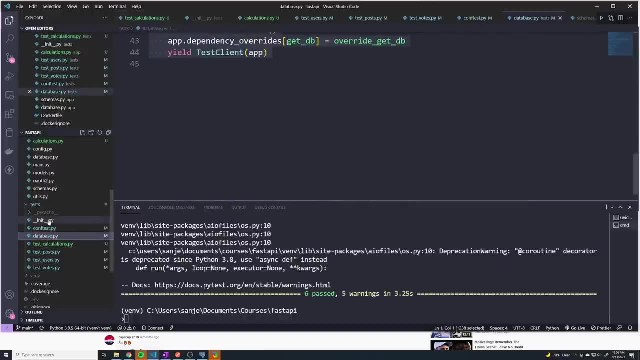 um, we don't need this test calculations py file, but i'll keep it in there in the repo just so you can take a look at it. the databasepy file is absolutely useless now, so i'm actually going to just delete. no, i'll just keep it there. 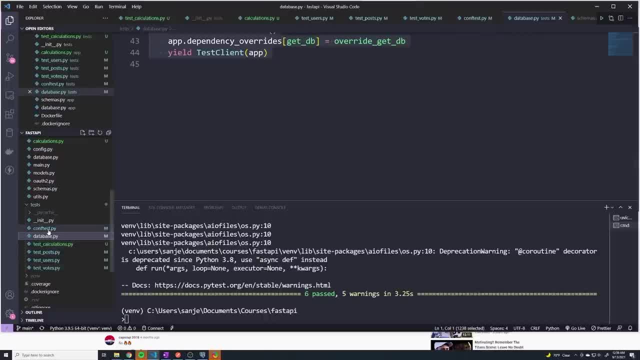 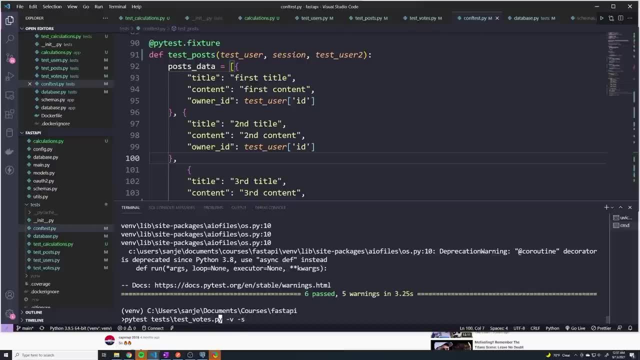 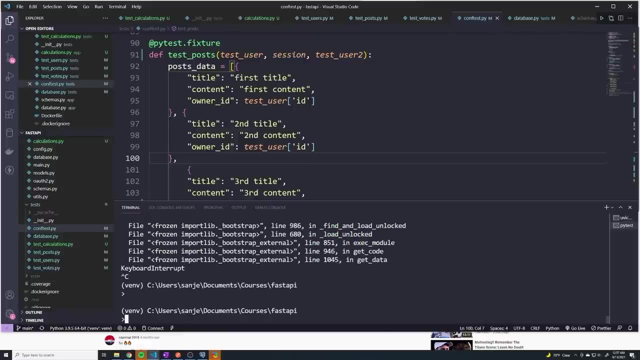 uh, just delete. I'll keep it in there, just in case you want to see it, But most of it's moved to conf testpy. But just to make sure that everything's still working, I'm going to run my tests for all. Oh, what happened here? Nope, nope, nope. Oh, okay, Yeah, that was wild. 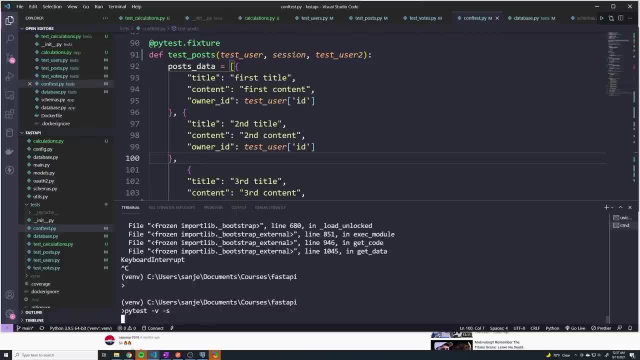 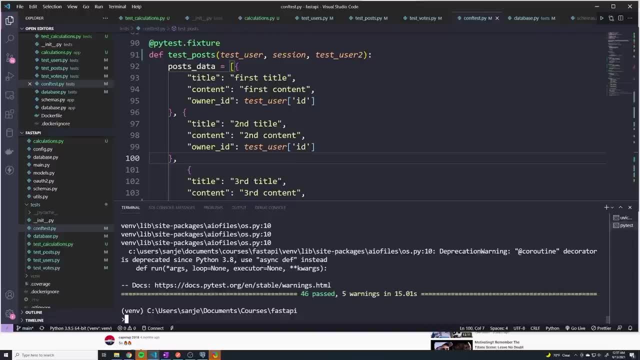 All right, Move this. Let's see what happens. Hopefully everything passes And all 46 tests have successfully passed. So that pretty much wraps up all of the testing section. I recommend you guys think of different scenarios that could potentially break our application. 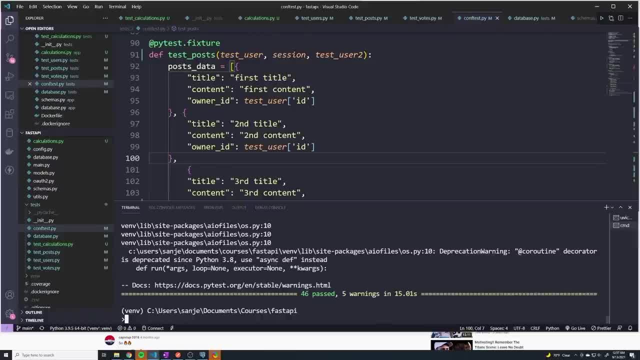 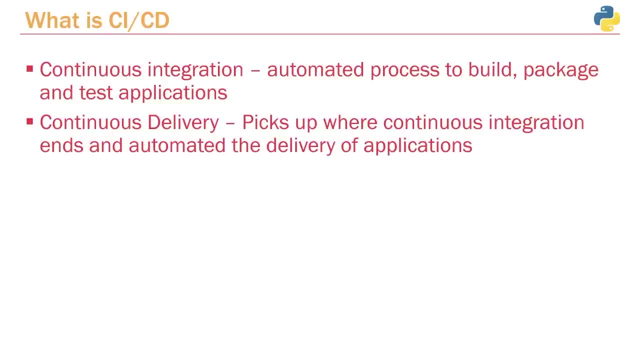 and set up tests for each and every individual scenario. Because that's how you successfully set up tests, because you want to make sure you cover every individual corner case that you can possibly think of. Currently, when it comes to adding in new features and making changes to our code, we have to go through a very manual and 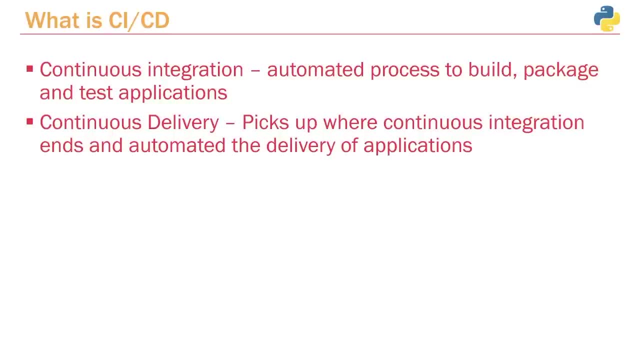 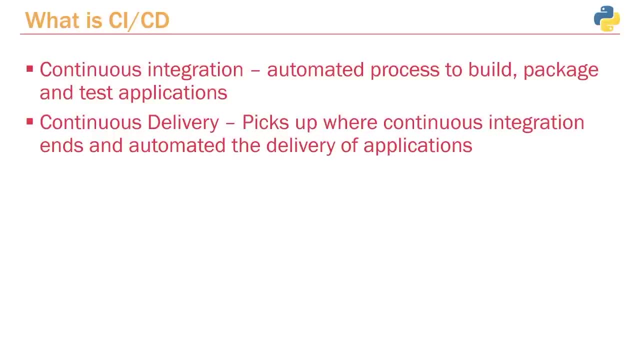 And so what I think would be good is for us to set up a CI CD pipeline so that we can do all of this in an automated fashion. So I've created a couple of slides just to kind of go over what our CI CD pipeline is going to do. And I've got the generic definition of CI CD And it's probably not a very 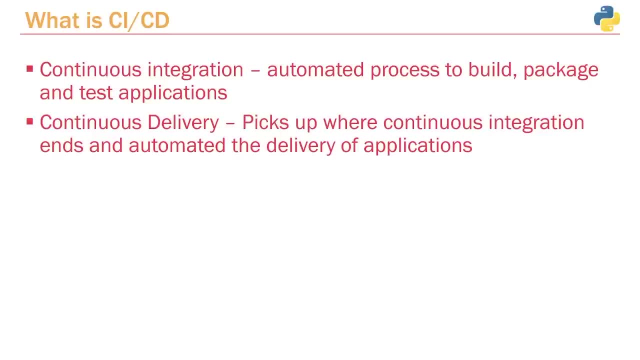 good definition And I was thinking about just leaving out the slide because it doesn't really provide much, but I figured I just added just in case. So CI CD stands for continuous integration and continuous delivery. So continuous integration is the automated process to build package and 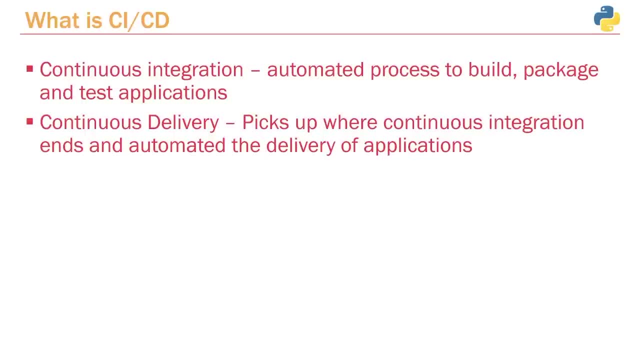 test your application And then the continuous delivery picks up where your continuous integration ends and automates the whole delivery of the application. So continuous delivery is responsible for actually pushing out those changes to your production network. So those two things make up our CI CD pipeline. But let's actually take a look. 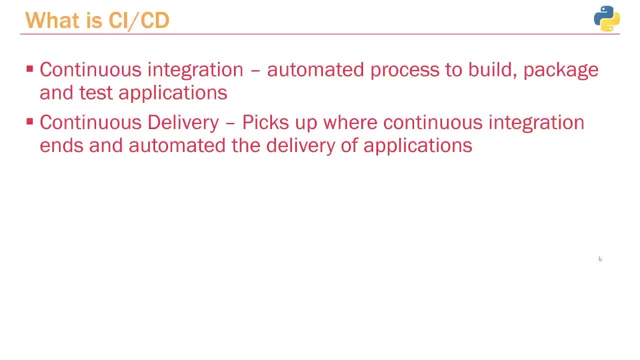 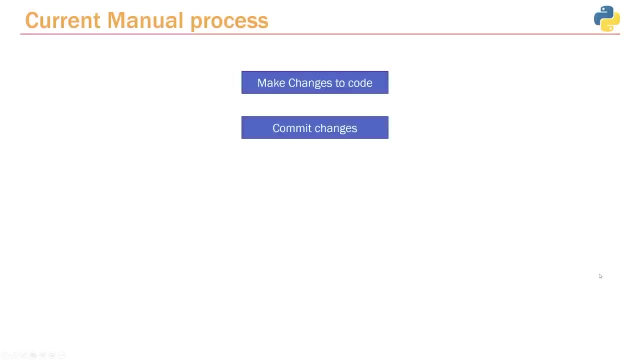 at what our whole manual process looks like right now, so that we can see where a lot of the extraneous time consumption and manual process takes place. So our current manual process is that you know we're going to make some changes to our code And then we're going to commit those changes to git, right, Because you know we don't want. 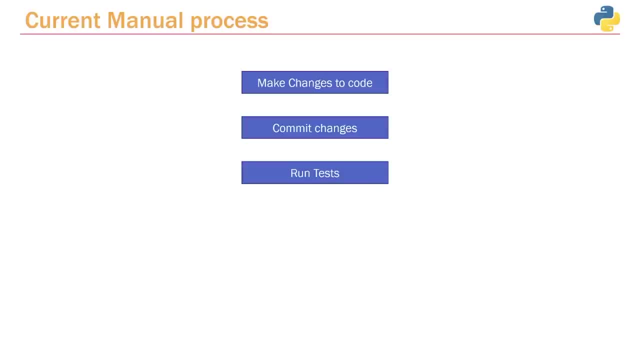 to lose those changes And then after that we want to go ahead and run py tests so that we can verify that our changes didn't actually break any known functionality to our code. And if our tests pass, we have an optional step of, you know, building any images. so we 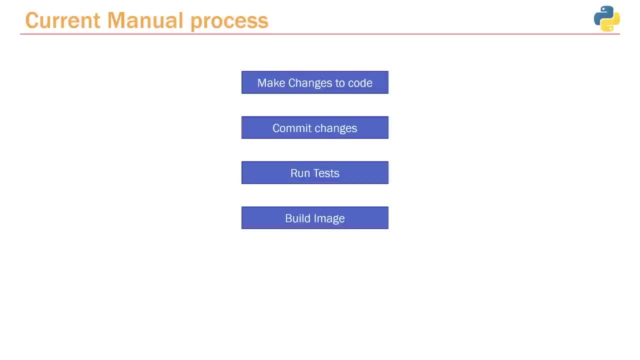 So things like Docker images, if we happen to be running Docker in our development and production environment. if we're not, then this is an optional step. However, when it comes to the build phase, in this case, that some people refer to, other, 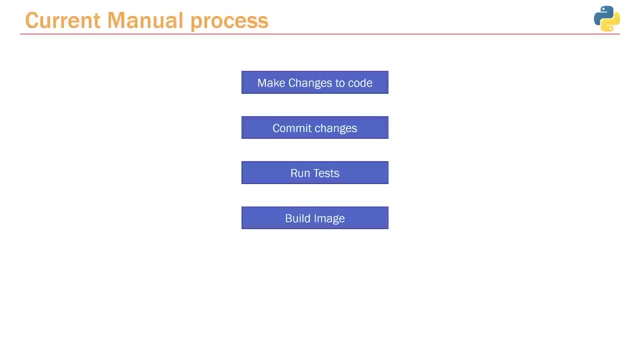 programming languages might require you to kind of build the application at the end to actually be able to deploy it. Python- you don't really need to do that, So that's why it's kind of an optional step here if you're not using Docker. 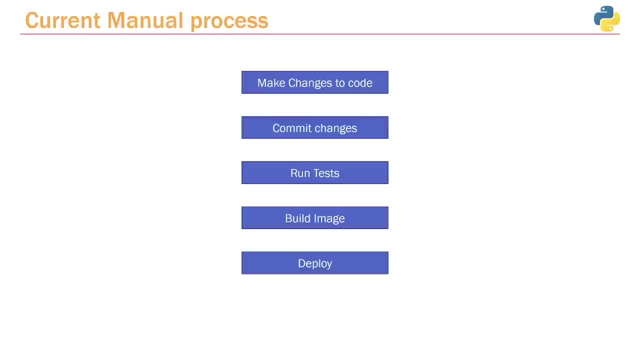 But after we do that we then move on to deploying our application. So I just have one row called deploy here. But keep in mind, this one little block could represent multiple steps because depending on how you actually deploy your application- making any changes or updating the code in. 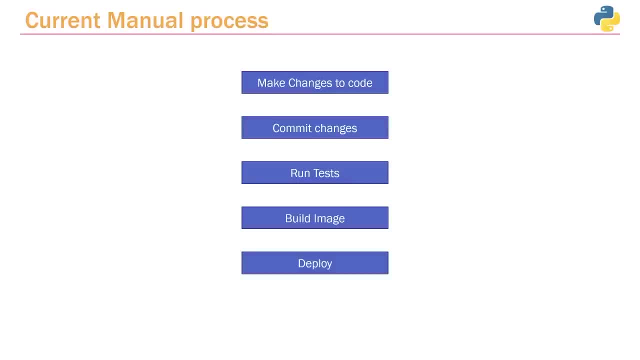 your production environment could actually involve a very complex process. So with Heroku it's obviously a very simple process because all we do is we just do a git push to Heroku And that's going to automatically cause Heroku to kind of handle all of the: the updating of the 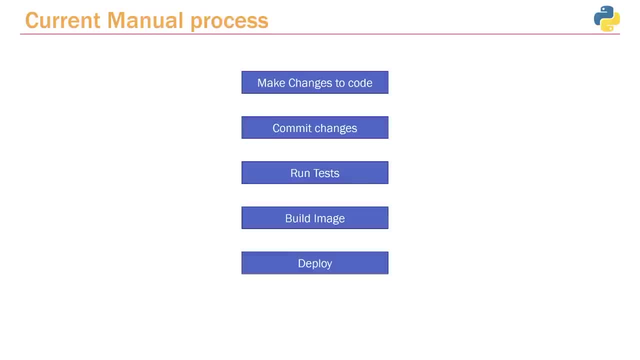 processes. So that's a feature that's built into Heroku, But we only get that if we use Heroku. there's obviously a number of different ways that we can deploy our application. If we decide to go the route of deploying our application on an Ubuntu server, then the 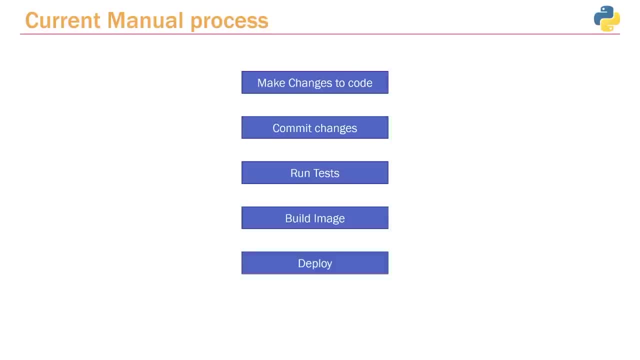 deployment process in this case would be us logging into our server, us pulling in the new code with the changes and then restarting the service so that our application actually uses the new code. But if you're using, you know- some other production environment or you use some other method. 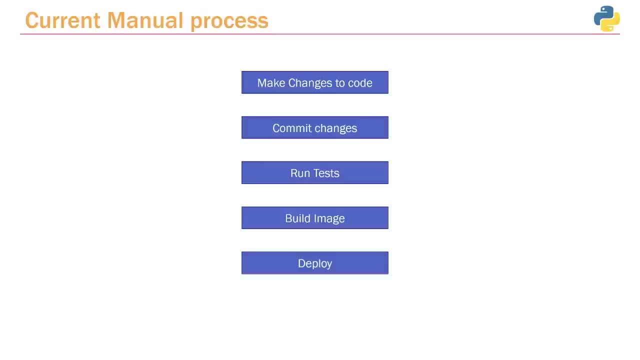 to deploy your application. this could be an even more complex process. Something to keep in mind. So, even though it's just one block listed here, it could actually be, you know, numerous steps. All right, And so now I want to show you guys what our automated CI CD pipeline is going to look. 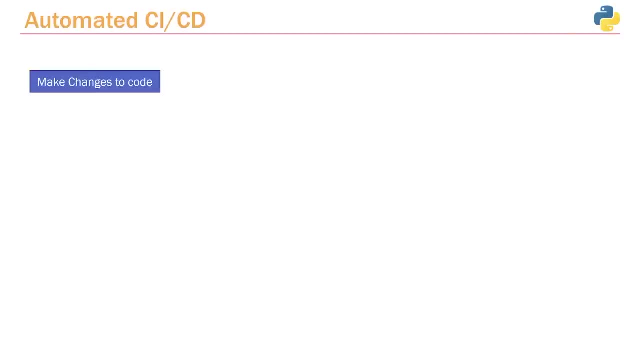 like after we set it up, And so, just like we did in the manual process, we're going to make changes to our code. Obviously, that's a manual step, because we have to implement the changes to our code, And then we're going to commit those changes. 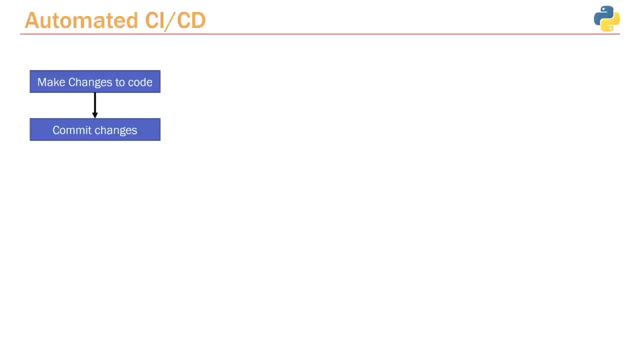 And with a CI CD pipeline, or specifically with the one we're building. that's all the manual steps that we have to do. We are done. We don't have to touch our keyboard or our mouse. It's basically hands off at this point. 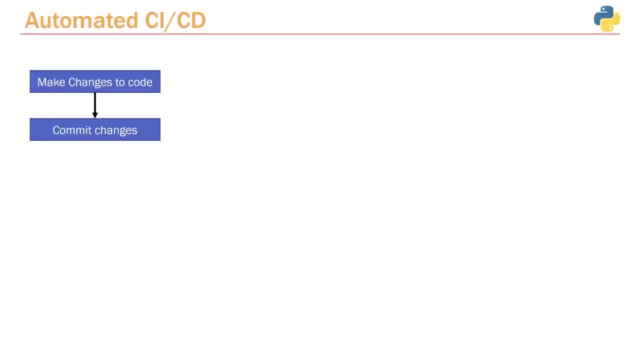 And we're going to let automation take over. And so usually, when you commit changes to your code, that's going to trigger our CI CD pipeline to run, And so what happens is our continuous integration phase starts At this point, as soon as we commit those changes. 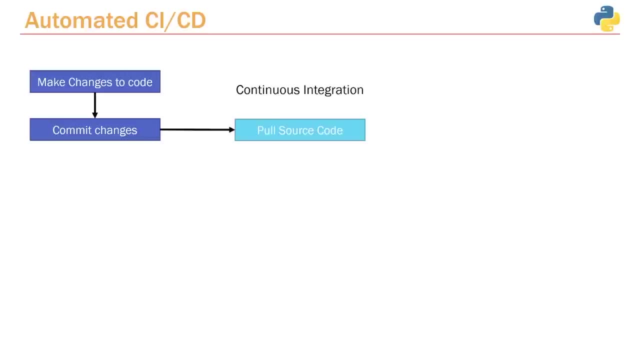 So in the CI phase we do the first thing that we do is we pull our source code. So we pull our source code so that we can actually work with it. We then install any dependencies. So this is the equivalent of installing all of the dependencies listed in our requirementstxt. 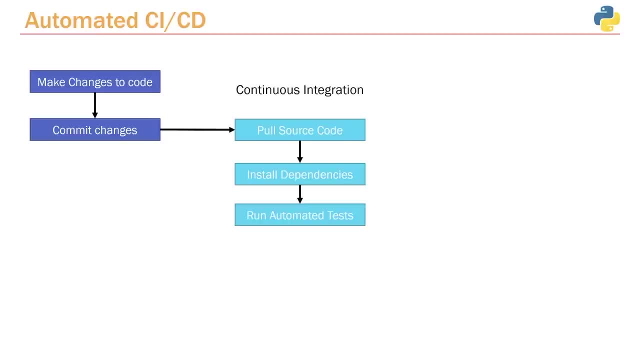 file. We then run our automated tests. So that's running PyTest, And then, you know, assuming the tests pass, we then build any images. This is once again an optional step for us. It's only in, that's only needed. 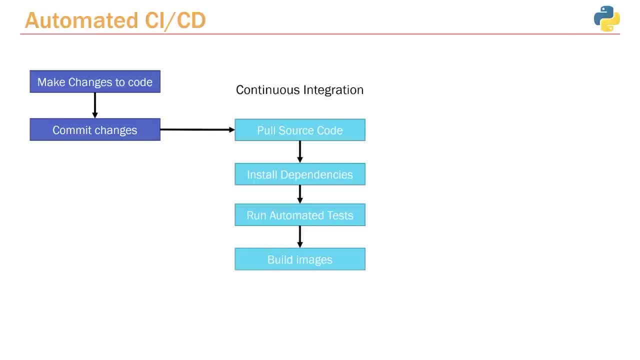 If we are happy if we use Docker. but that wraps up the continuous integration phase. So once that's done, the continuous delivery phase is going to take over, And so the continuous delivery phase. what it's going to do is it's either going to grab the 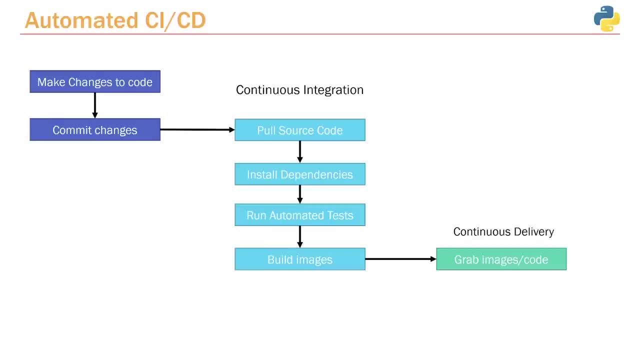 latest code or the new build image, depending on what our deployment model actually is, And with the new image or code it's going to then have all of the logic needed to push that new image or the new code into our production and make sure that our production is actually 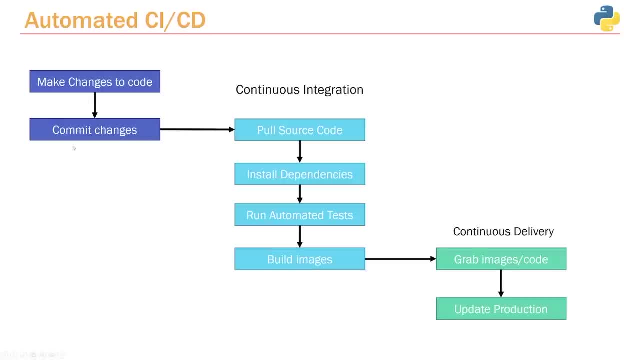 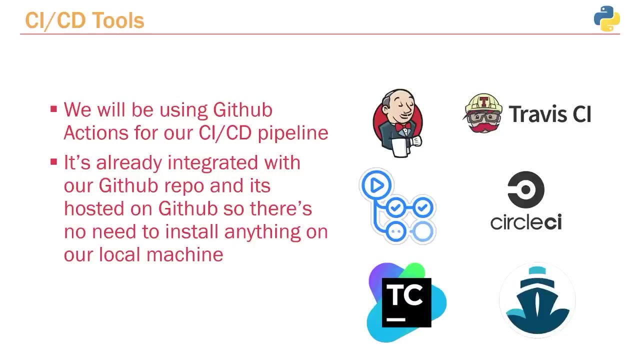 using our brand new code, And so these two steps are really the only manual steps can be. continuous integration in the continuous delivery phase is all done in an automated fashion, through code essentially, And so some of the more common CI CD tools include Jenkins, Travis CI, Circle CI and GitHub Actions. 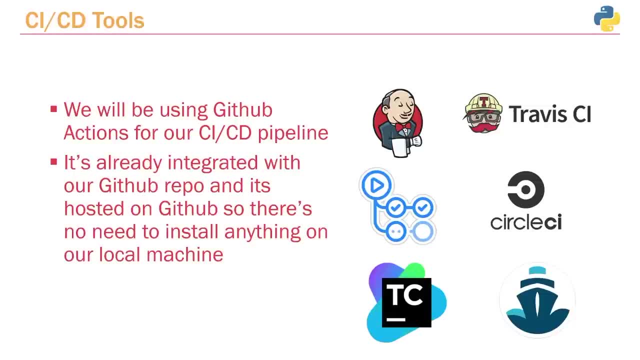 Now for our course. we're actually going to use GitHub Actions just because it's already integrated into GitHub. It's free. We don't need to install anything on our local machine. There's no software that we have to set up, because it's all hosted on GitHub. 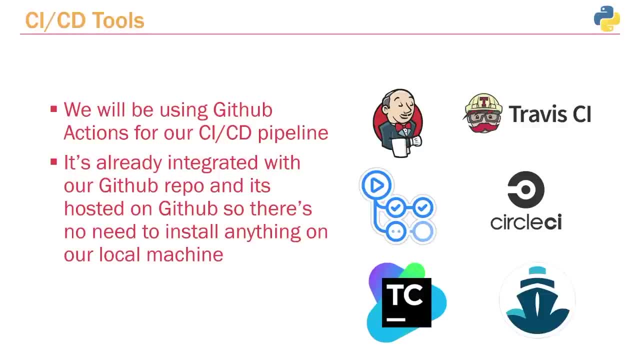 So it's like a hosted service and it's just going to make things very clean, very simple, And it's free, So it's going to make and so everyone will be able to have access to it. So what exactly is a CI CD tool? 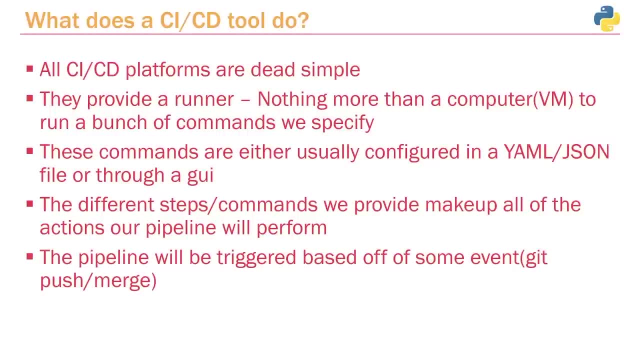 What does it provide? And so every time I heard CI CD before I learned what it is, I always thought it was a very complex thing. And then, when you find out what it actually is, it's actually this stupidly simple. there's no magic behind CI CD. it's all very manual, even though it's an automated process. 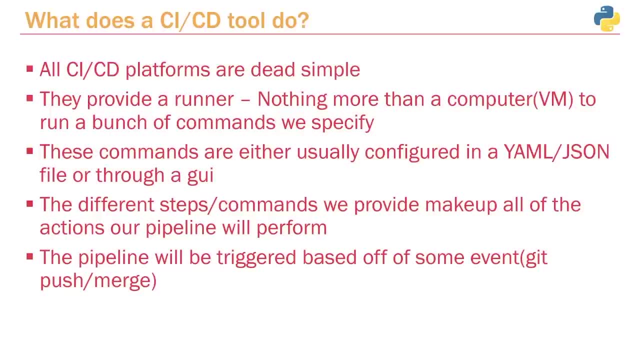 You'll see that when we actually go to configure it, it's not really doing anything special. It's doing everything that we already do, but we're just providing instructions to a machine. So a CI CD tool. what it does is it provides us a runner. 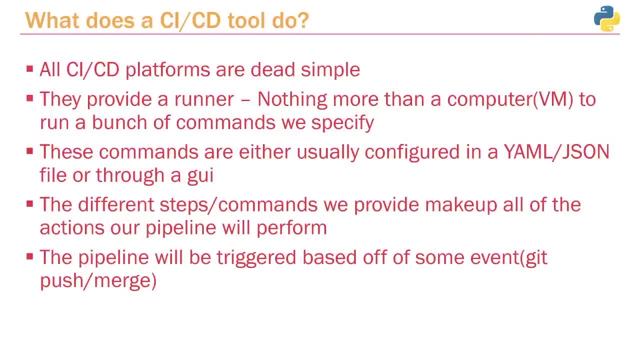 And so a runner is just a fancy term for a computer or a virtual machine. It doesn't really matter. You know what is the underlying infrastructure. They give you a little machine That we can provide a bunch of commands for it to run right. 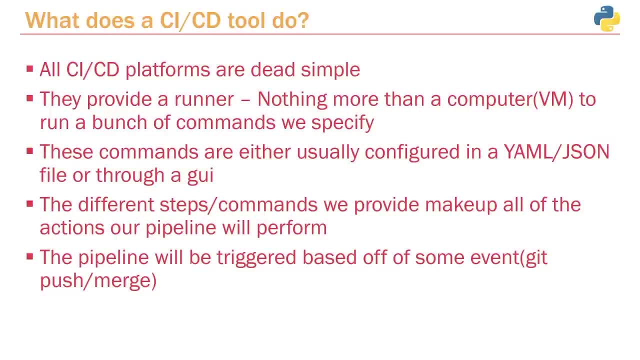 So, just like in our terminal, where we run commands like pi test or or pip install right, We provide these commands to a computer, and these commands are usually configured or provided in a YAML or JSON file or even through a GUI, depending on what your CI CD tool is. 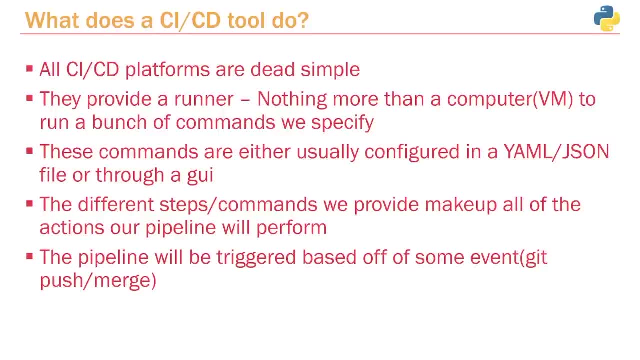 But the different commands that we provide that little mini computer to run make up all of the actions that our pipeline will perform. And this pipeline, Or this virtual machine that we have, is going to run based off of some event getting triggered. And so, like I mentioned, this is usually us either doing a get- push or performing like a merge pull, a merge request. 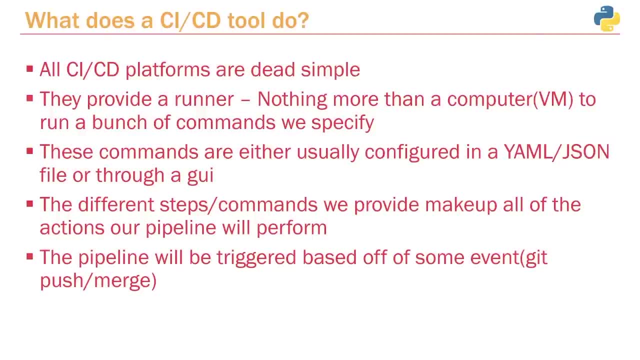 It doesn't really matter. There's a lot of different events that you can configure depending on your CI CD tool. You can also set it up to run every single night at two in the morning. There's a lot of different options, but mostly it's going to be based off of a get push. 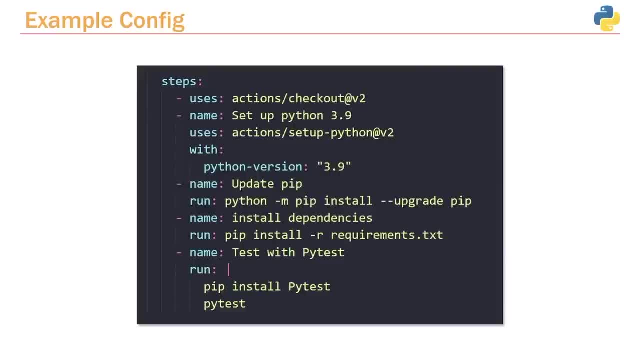 And I wanted to provide just a quick example config of what our CI CICD pipeline is going to look like when we're done. So this is just a little snapshot of it. It's not all of it, but I wanted to show you just how simple setting up a CICD pipeline is. So this: 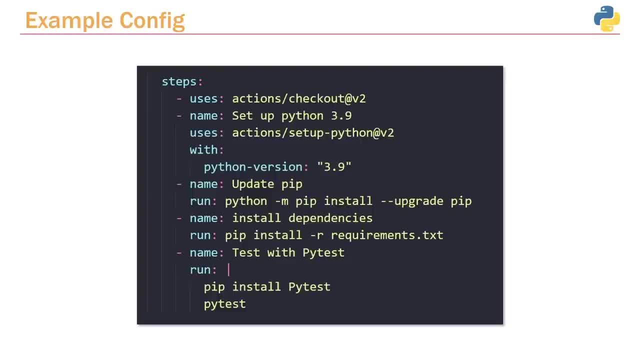 is the YAML file that we use to kind of tell the machine what are the steps that we want it to perform, And so you can see. here we've got this section called steps, So already you can tell. we're just providing it a list of steps. Now the syntax may be a little foreign, but you'll see. 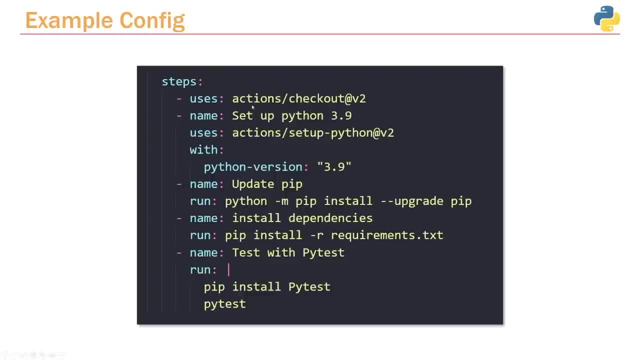 that it's pretty easy to learn. You'll see that the first step that we have is there's this thing called action slash checkout. So what this is actually doing is it's telling our machine to pull our code. So after we do a git push, it's going to pull our brand new code so that we can. 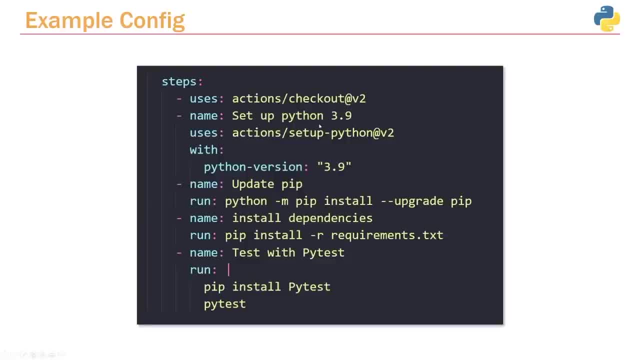 actually do something with the code. And then the next step is: here we're setting up Python 3.9.. So all it's doing is it's installing Python 3.9 for us, And then afterwards we have to update pip. So it's going to run python-m pip install dash, dash, upgrade pip. So that's going to upgrade. 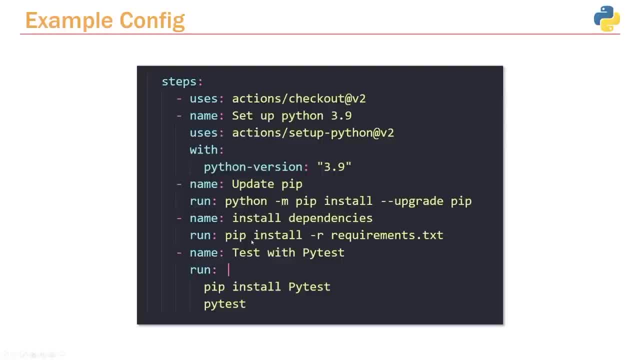 pip, So we have the latest version. Then we're going to install the dependency. So that's pip. install dash r requirementsts. So you can see all the things that we do on our local machine. we're just telling this little machine to do the same thing And then afterwards we then run a pi test. So that's going to first. 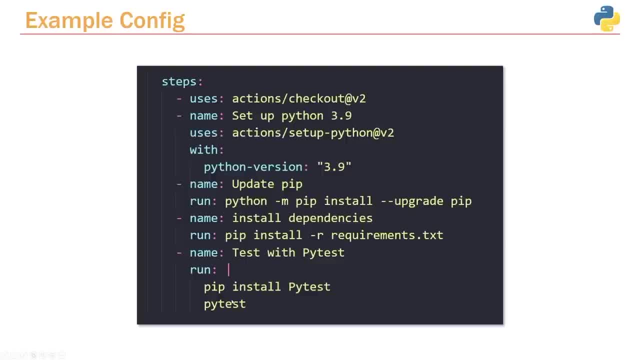 install pi test And then we just run pi test, right, Just like we did on our local machine. we're just telling the machine to do the same exact thing. So we're just telling the machine a list of instructions that we have done by ourselves manually. We're just giving that. 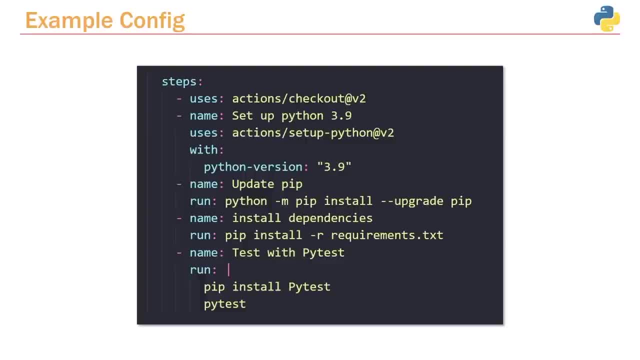 list to it so it can run automatically, And so hopefully, you guys see just how simple a CICD pipeline is. There's nothing magical to it. It's just like telling a machine. this is what we want to do. I want you to run this every single time we do a git push. 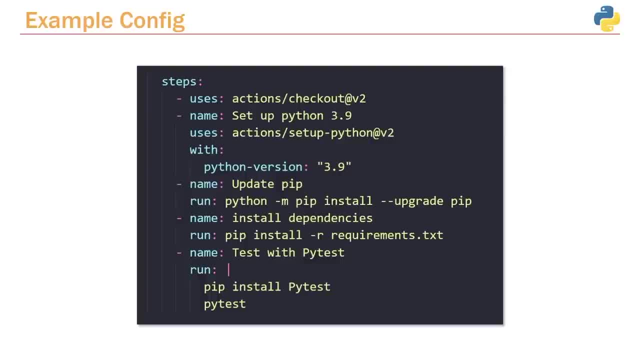 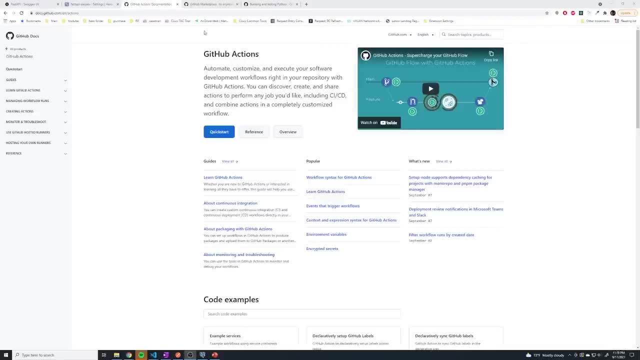 All right, So hopefully you guys understand this. In the next video we'll get started on setting up GitHub actions so that we can actually build out our CICD pipeline. All right, before we get started with working with GitHub actions, I want you to open up a couple of web pages. 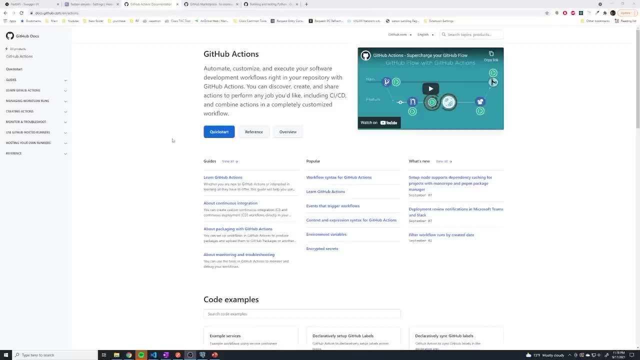 So if you go to the GitHub actions documents page, I definitely recommend you pull this up. Take a look at the quick start page and the reference page just to get an idea of how to work with GitHub actions. I will cover everything, But you know you are going to forget some things I cover. 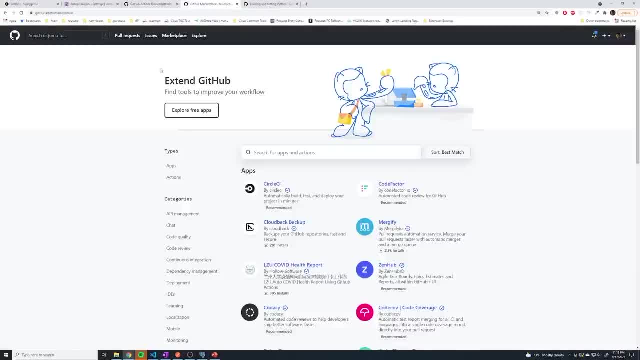 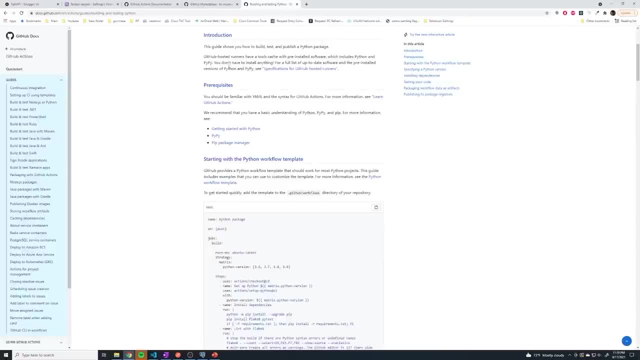 So definitely know where the documentation is. Pull up the GitHub marketplace as well. So this is where we can look up built in actions that we can use in our CICD pipeline. that have kind of handled a lot of the more complex logic. And then on top of that you'll see that GitHub has this example tutorial on how to set up a CICD pipeline for a Python application. 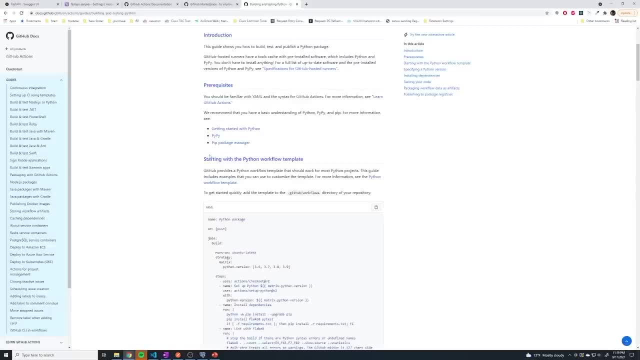 So this is what I kind of looked at to get started with building out a CICD pipeline- pipeline for our fast API- And it kind of covers most of the things we do that we need. So if you want to, you could just follow this And I think at that point you'll have a good idea as to how. 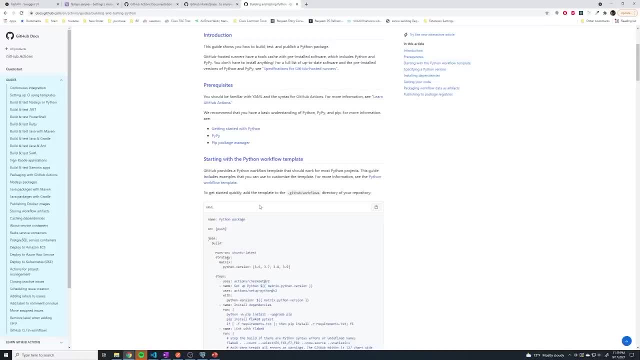 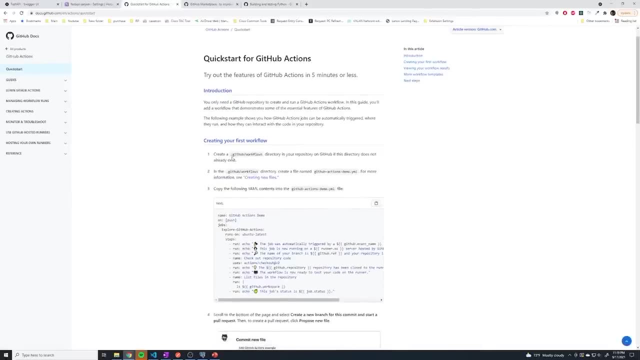 to work with this. But once again, like I said, we're going to cover everything from scratch. But if we go to the documentation, you go to quick start right here it tells you that we want to create a folder called GitHub And then in that folder, 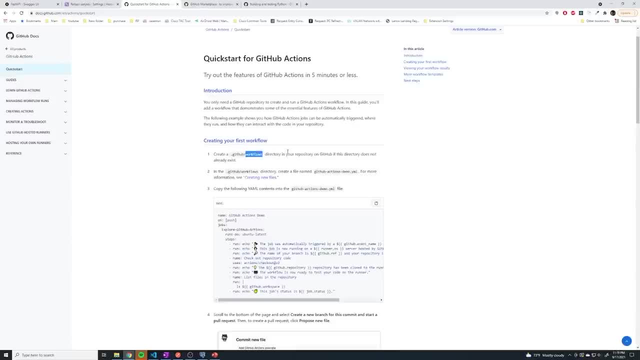 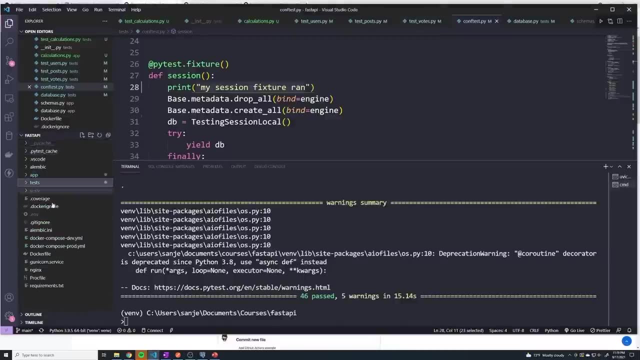 we want to create a folder called workflows, So let's go ahead and do that. So in our main project directory- let me just minimize everything- I'm going to create a brand new folder And I'll call this dot GitHub. And then we want a new folder within here called 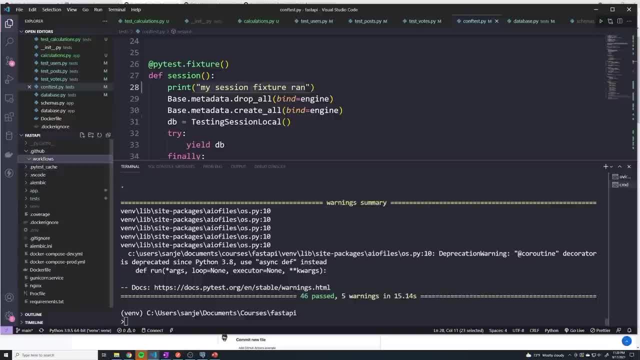 workflows, All right. and so here we can define all of our workflows which kind of make up our CI CD pipeline. you can have more than one, you don't need to just have one in this case, but we're just going to use one because we're keeping things simple. And so here, this is where we're. 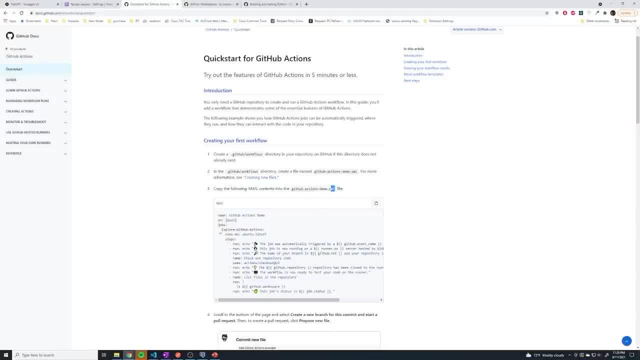 going to go ahead and create a new folder called workflows, And then we're going to go ahead and create a YAML file. So if you aren't familiar with YAML, it's just a certain type of markup language that's commonly used for like config files and things like that, because it's very 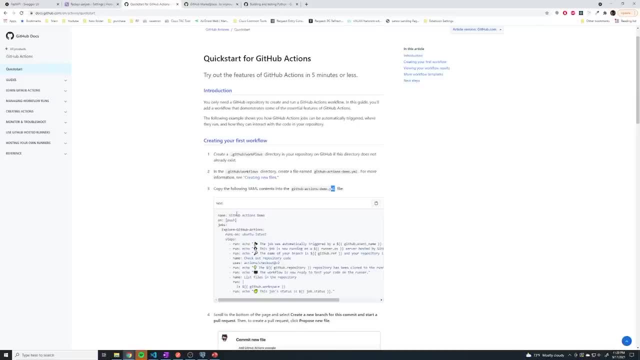 easy to read, But the most important thing to keep in mind is that spacing matters in YAML, So you definitely want to make sure that all the things are lined up very carefully, just like it was when it comes to like the Docker compose file. So we'll go here. 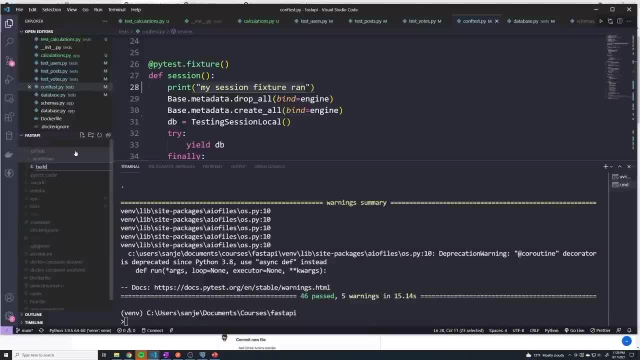 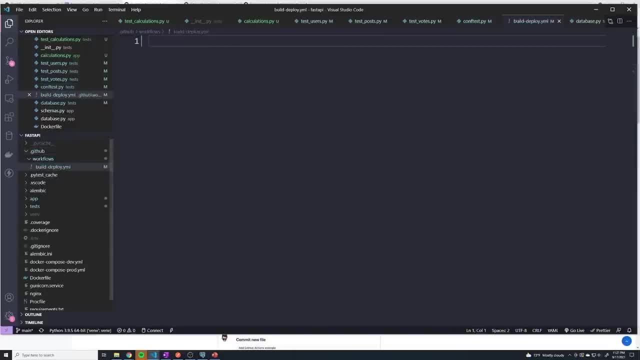 and I'm going to create a brand new file And I'm going to call this build dash deploy dot YAML. All right, and so we're going to give this workflow a name. So even though we gave it the file a name, we actually have to provide a name here. So we just do name and feel free to. 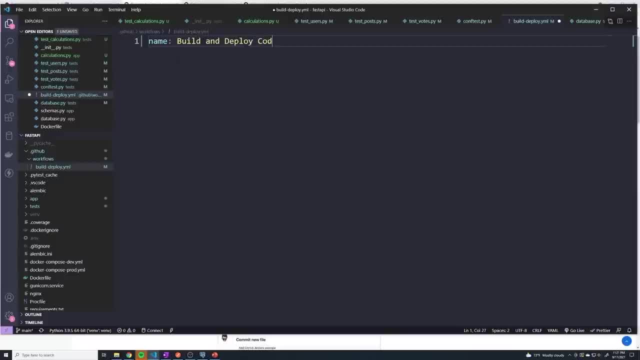 call it whatever you want. I'm just going to call this build and deploy code. Okay, and then we have to define when should our workflow or, in this case, which is our CI CD pipeline, when should it run, When should it trigger? What triggers our code to run? And so, like I mentioned, it's usually a 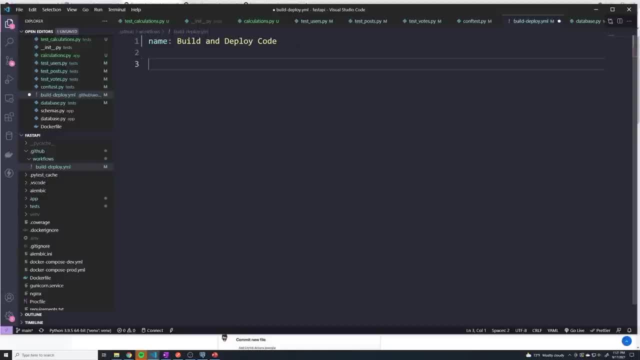 either a pull request or a get push. So to specify when we trigger this, you pass in the on field And then you specify, you know, should this be a push or a pull request, Or should it run for both? And so if you want this to run only on get pushes, you would just do on push. 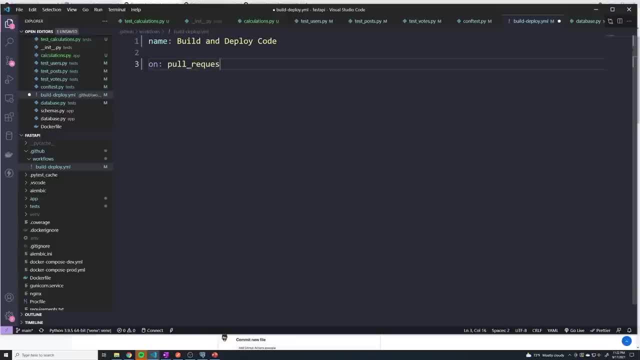 If you wanted to run on pull request, you do pull request here. But if you wanted to run for both- get push and pull request- then you would do push and pull request, And there's a lot of flexibility too. So the way we have it set up right here, this would happen on every push on. 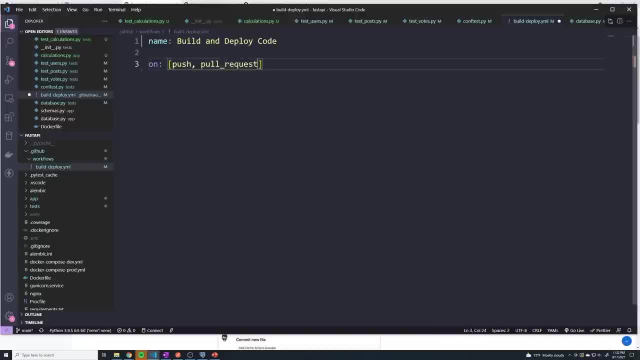 every single branch and every pull request on every single branch. but there's a possibility that maybe you don't want this to run for all of your branches, Right? Maybe you only want this to run on the main branch and a couple of other branches and then the rest of the branches you 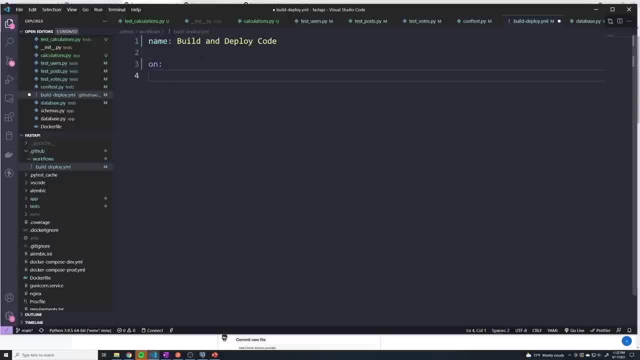 don't really care about. So what you can do is we can go down a level And then you can get a new one. then hit tab in this case And remember, like I said, spacing matters. So we'll say push. 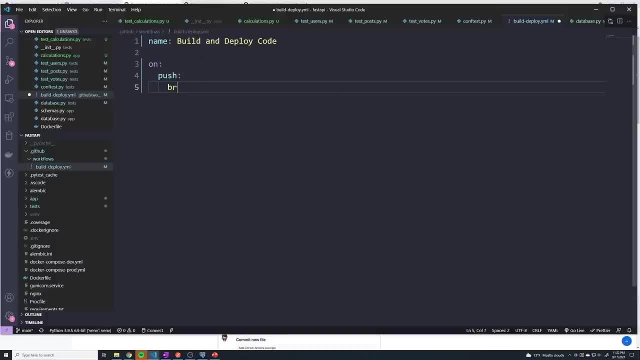 And then here you can define all of the branches that should run whenever you do a push. So if I here, I pass in main. what's going to happen is that this workflow is going to trigger, every time we do a push, specifically only to the main branch and no other branches. 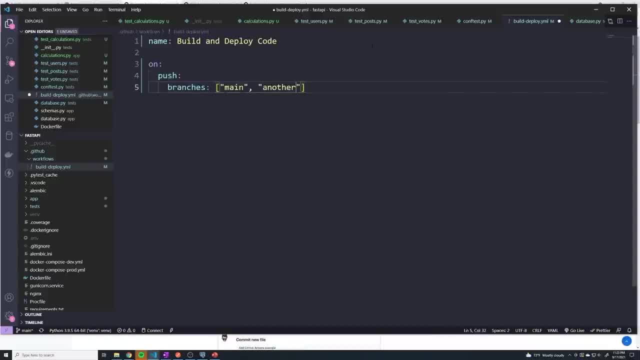 And so you can provide a list of all the branches. So this is, you know another branch. This is, you know, maybe some feature branch- all the names of the branches that you want your workflow to run on. you can specify that And this is one way of providing a list in YAML. 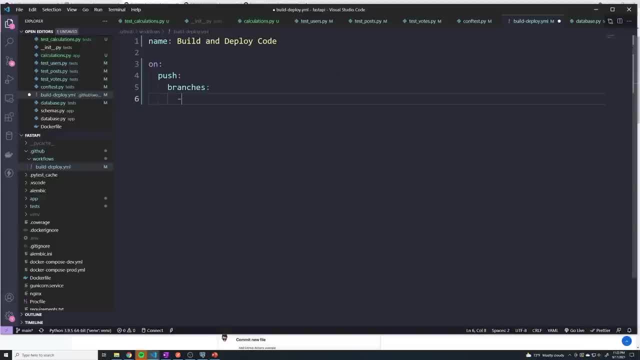 The other way is to actually go down here and then do a dash and then provide the name. So I would do main, And then you know some other branch and so on, And then, if we wanted to, we could also customize all of the branches that. 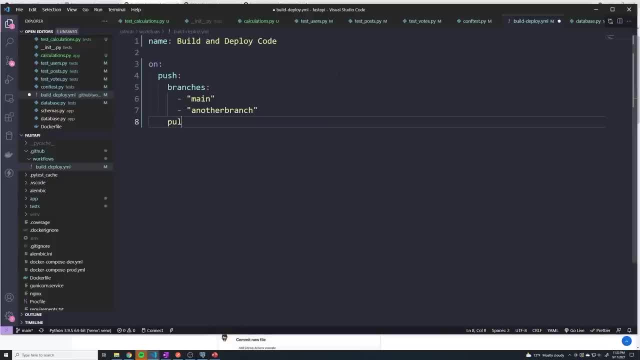 should trigger this workflow on a pull request as well. So if I do pull request and then I do branches and this should be moved back here And then here I do branches And then I can do a list here as well And I'll just call this. we'll give an example: branch. 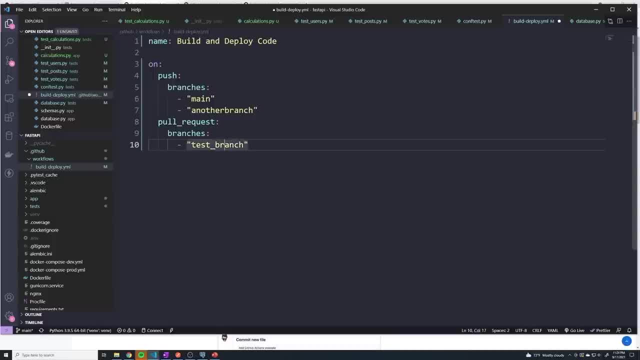 I'll say test branch Right, And so just to kind of read this through: anytime we do a push to either one of these branches, we're going to be able to do a push to either one of these branches. It's going to run our code And anytime we do a pull request to this specific branch. 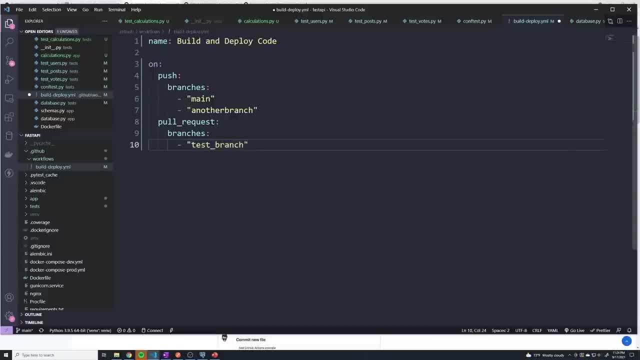 it's going to run our code as well. So that's just how to set this up. we're not going to do any of that because we just have one branch in this case. So I'm just going to say we're going to. 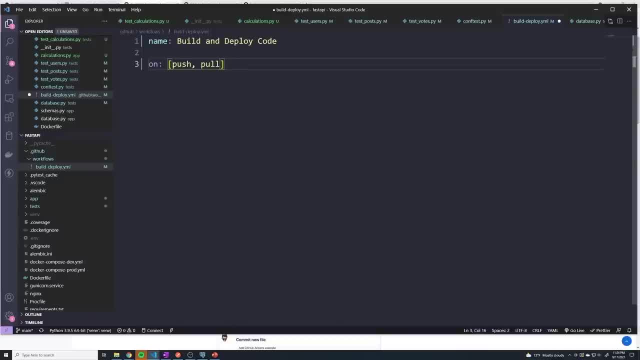 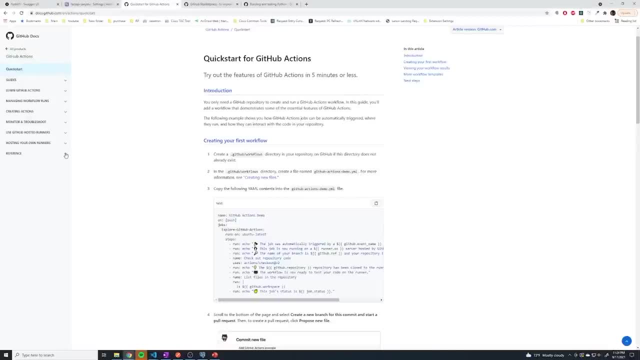 run this on push and pull requests for all branches And if we actually go to the documentation, I think, yeah, the reference page. you can go to the reference page and then select events that trigger workflows. So if we go to the reference page, we can go to the reference page And then 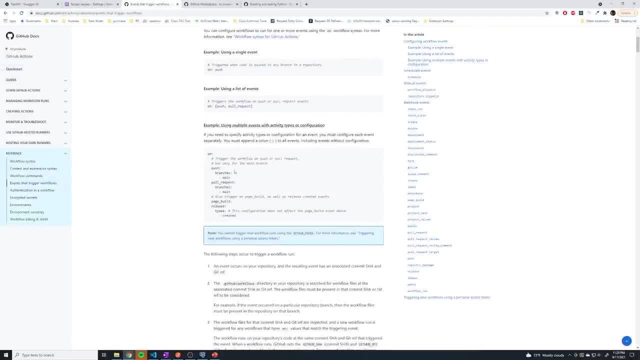 It's going to run our code and any time we do a pull request to this specific branch, it's going to run our And that's going to cover everything that we just covered. So it's going to go over all of that And you'll even see that there's a scheduled event. 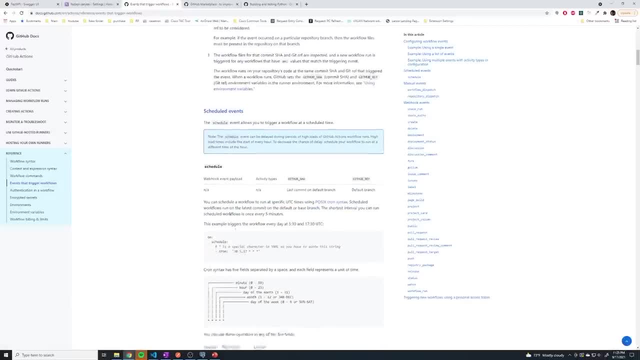 So you can tell it to run kind of like a cron job, Like hey, I want this to run every single hour, And there's a few other like manual events that you can trigger and a couple of like webhook integrations as well. 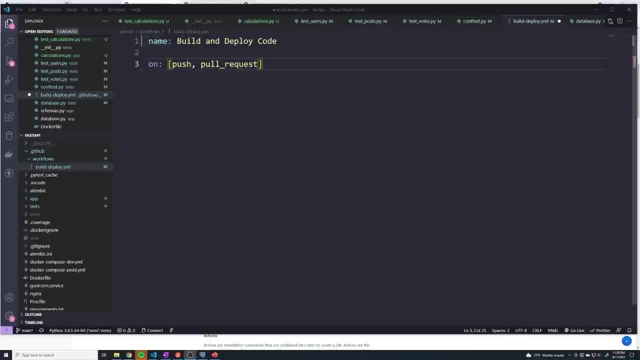 But we're not going to do any of that. We're just going to keep things simple for now. All right, So once we've defined what's going to trigger our workflow, we have to then create a job, And so if you go to the documentation, the GitHub actions documentation says that a job 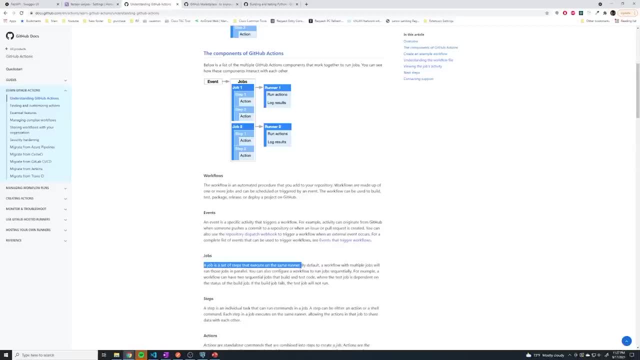 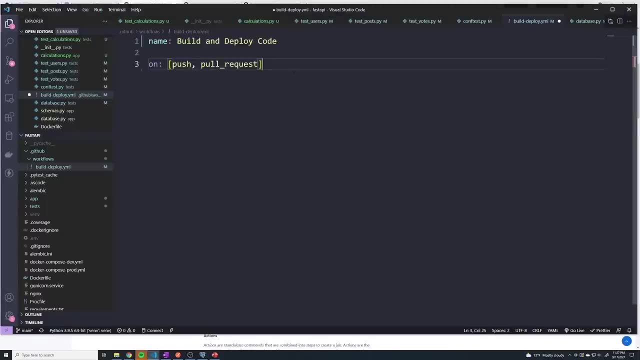 is just a set of steps that execute on the same runner. So our runner is just a virtual machine. So when our workflow runs, it's going to, we have to provide it a job, which is just a list of steps that's going to run on that specific runner. in that case, 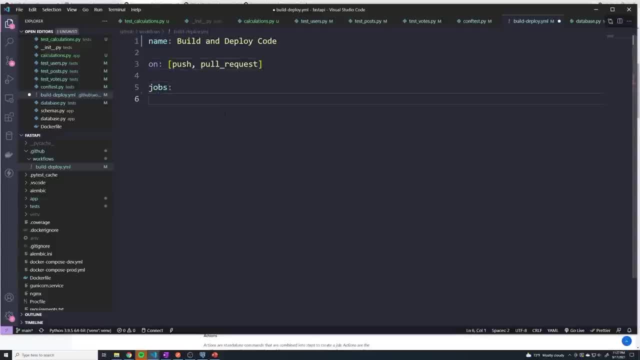 And so here I'll go to jobs. This is where we provide a list of jobs. We're going to start out with just one in this case, and we can give this whatever name we want. I'm going to call this job one, not a very good name. 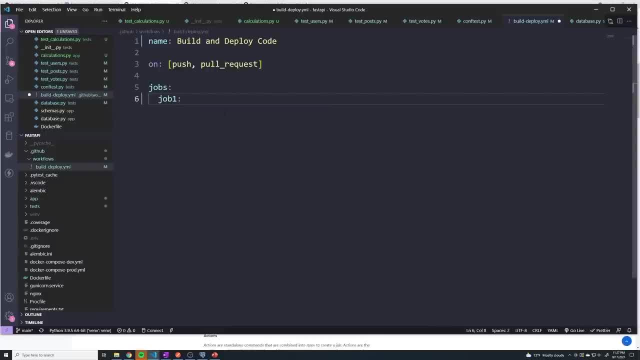 We're going to rename it in the future, But I want to just keep it simple for now. And what we want to do is we want to specify what type of machine do we want to run this on, And so, like I said, a CICD tool like GitHub actions is going to provide us a machine. 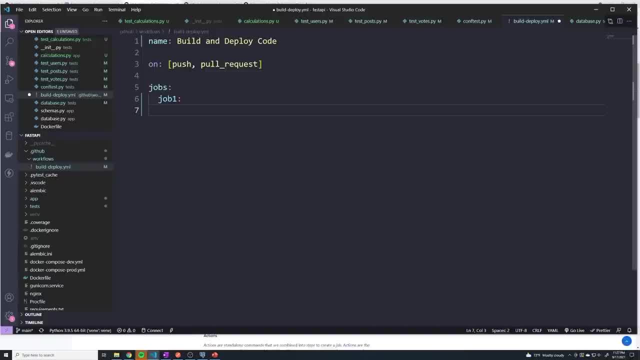 a computer And we have to specify what operating system do we want to run it on. So we're going to just use it on on Linux. But keep in mind, you can run this on Windows, You can run this on Mac. You can even run it on all three if you want to test all of them. 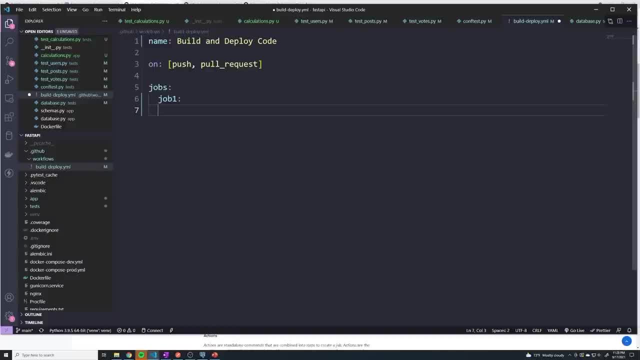 But since our deployment All right, Since our production environment is running on Linux, I think it makes sense that we do all of the testing and all of this on a Linux machine. So you pass in the runs on field And then here we say: Ubuntu latest. 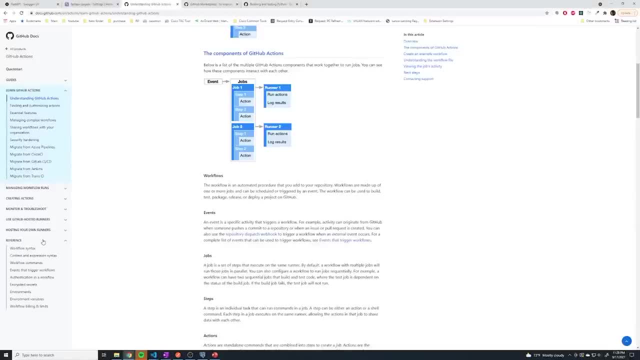 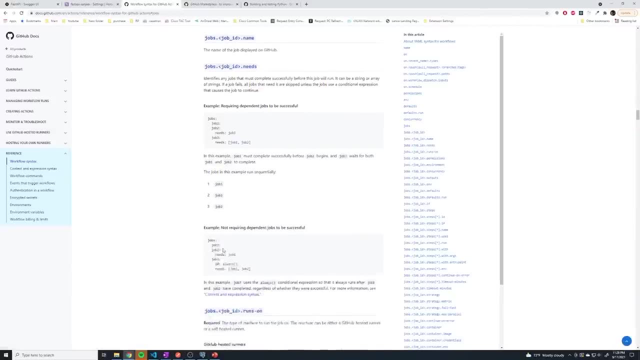 So this is going to be the latest Ubuntu version And if we go to the reference page here and go to the workflow syntax, I think, and we go to jobs, that's going to provide us all of the information when it comes to what we 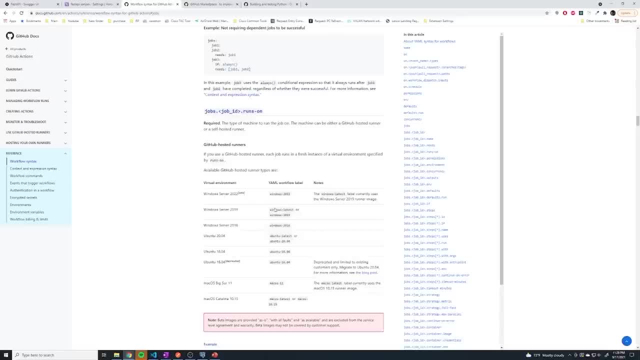 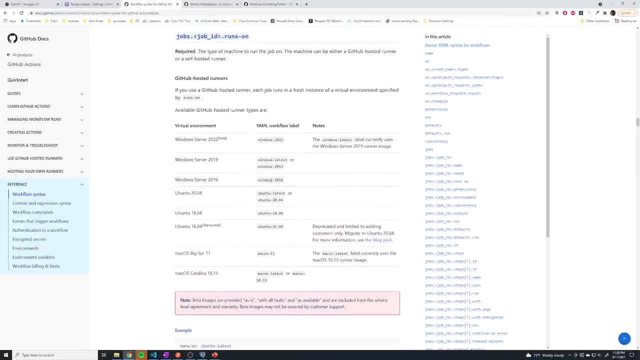 can run this on. So you can see, here we can provide Windows 2022 or you can just grab Windows latest. We've also got- And I realize the text is probably small for you guys- We got different versions of Windows. We got Ubuntu latest, which in this case, at the moment, is just going to be the same thing as 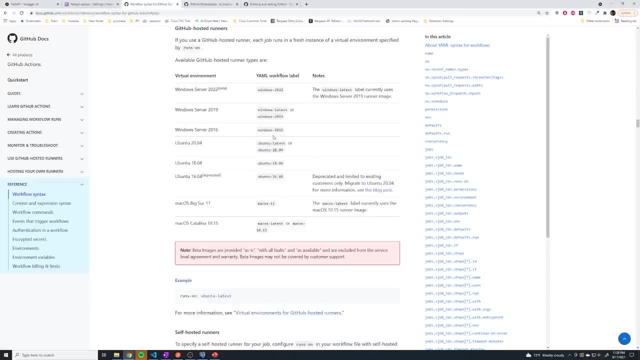 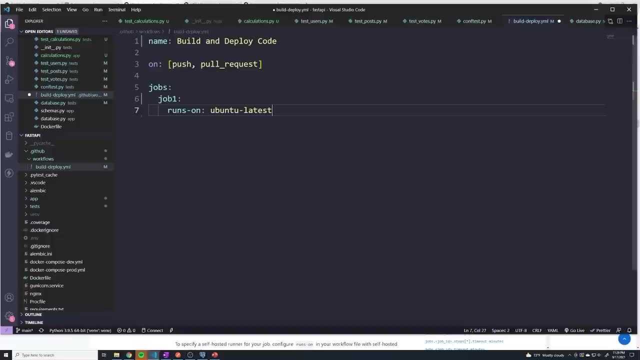 writing Ubuntu 20.0.4.. But you can grab any one of these specific Ubuntu versions, as well as Mac OS 11 and some of the other previous Mac versions. But, like I said, we're going to stick to just running on Ubuntu and we might as well just grab. 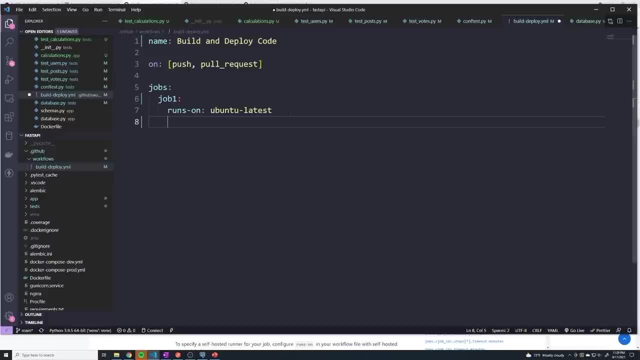 the latest version. And so once we specify the operating system, the next thing that we have to do is provide a list of steps. So we kind of Went over what the steps would look like when we did the little PowerPoint demonstration. So we here, we say steps. 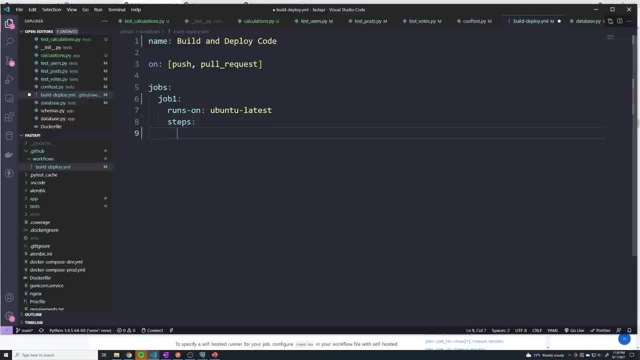 And then we provide a list of steps. So when it comes to lists in YAML, you just do the dash and then you provide the list, And usually when it comes to a specific step, we give it the specific command that we want to run. 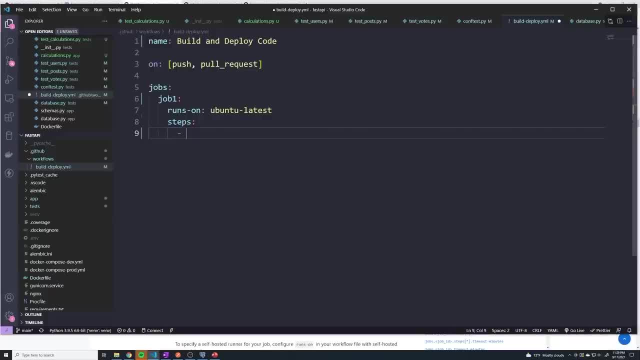 as well as a name, a human, readable name, so that when we look through the logs we know which step is doing what. So we can say like, hey, this step is installing Python, Or this step is running PyTest. And so here we say name. 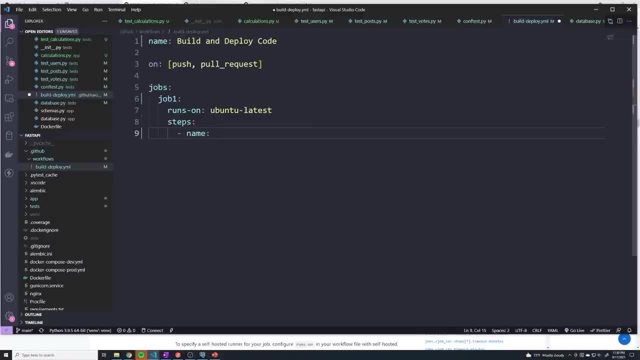 This is where we provide a description for what we're about to do. So the first thing that we always want to do is we want to check out our code, And so I'm going to say, hey, this is checking. Or I'll just say: this is pulling Git repo. it's going to pull our code, and then we have to provide the uses. 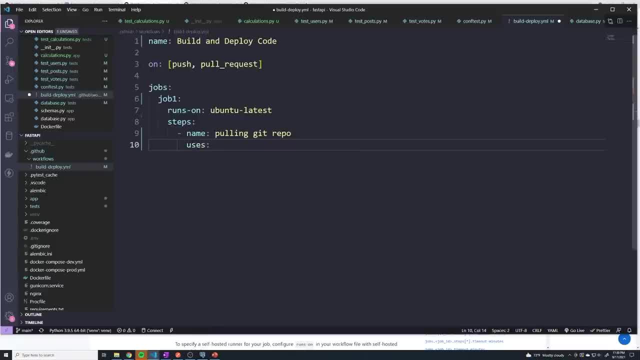 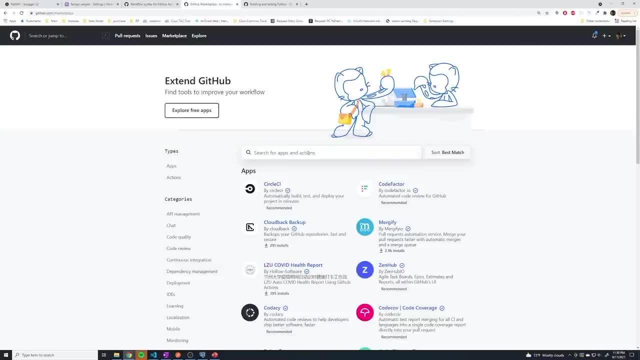 So this is the actual command that needs to run on our machine to pull our repo. And with GitHub Actions, like I said, there's a marketplace of pre-built actions that we can use to essentially perform various tasks, So pulling your code is a very common task. 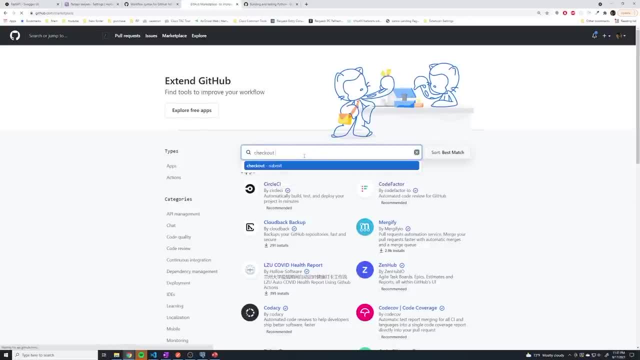 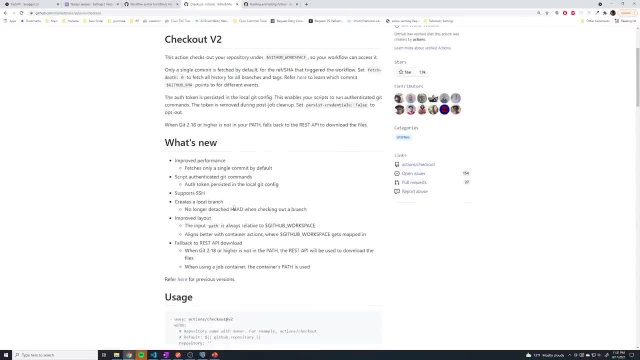 So they've definitely got an action for this, And so if I just search for checkout- because I know that's what it's called- you can see this is the one we want, And so this is this is what's going to be responsible for pulling your code. 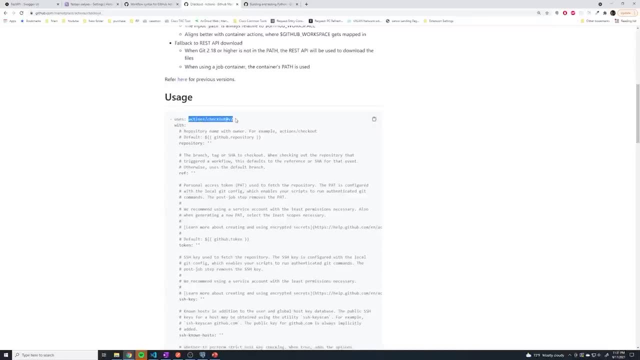 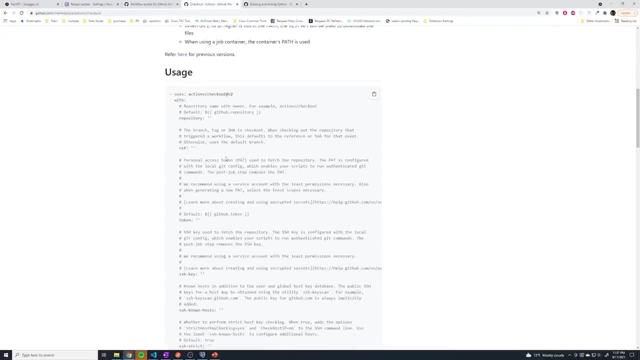 And so here you just say uses, you do actions, slash, checkout, v2.. And you could specify a specific repository that you want to pull. However, GitHub already knows what repository we're working on, because we did a Git push And since all of this is integrated together, we don't actually have to pass in any other field. 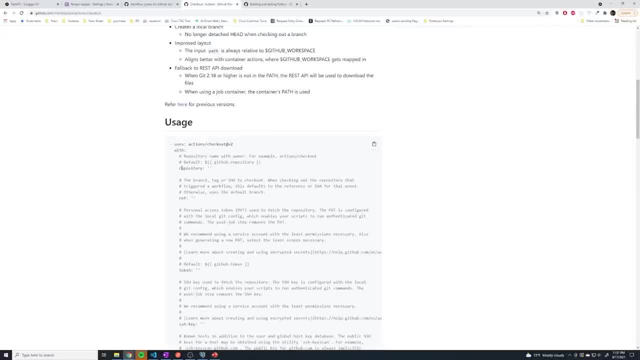 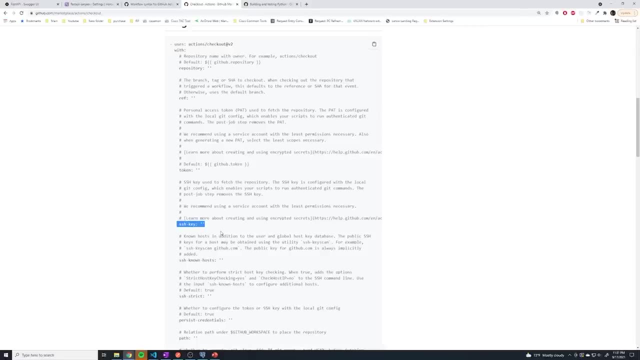 However, you know, if you look at the documentation, you can specify what specific repository you want, as well as you know any SSH keys that you may need and things like that. But this is GitHub Actions, So it's all already hosted on GitHub. 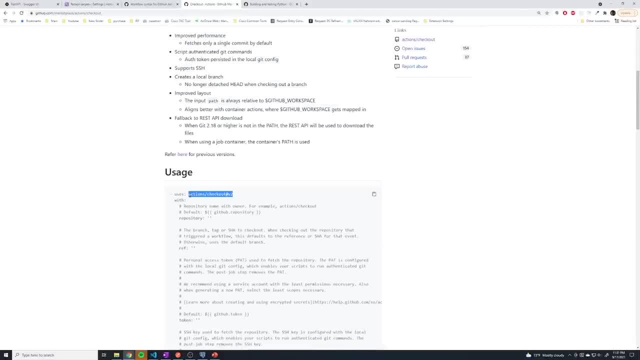 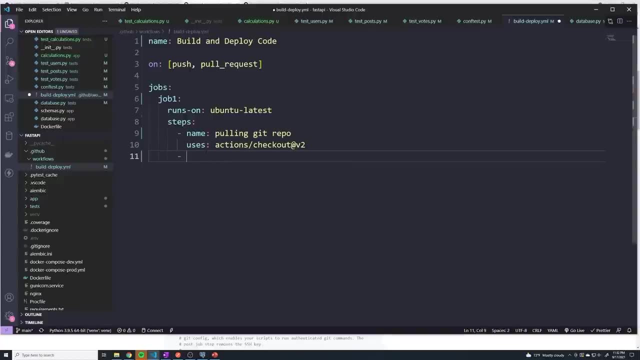 So it's a pretty simple. It's a pretty simplified process. So all we have to do is just copy this right here And we can just kind of continue down and just provide as many extra steps as we want. I'm just going to provide a very simple step after this, just to show you. you know, a step is just nothing more than us giving a command. 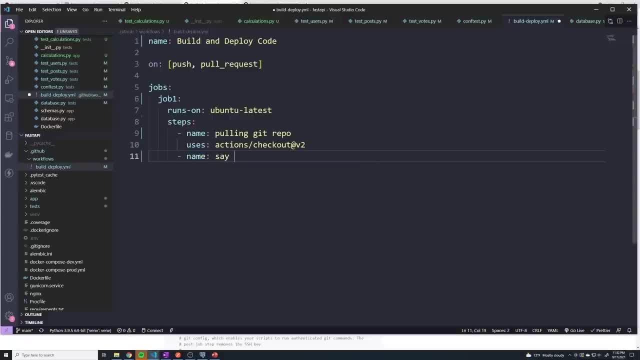 So I'm going to name this one, Say hi to Sanjeev. And what we can do is: this is a special action, that's that we grab from the marketplace. But if you just want to run a command on the machine, which is just a Linux machine, 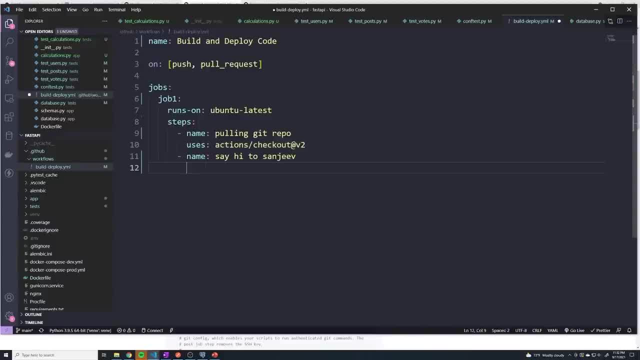 run any specific Linux command that we want, because we have access to the CLI. all we have to do is just use the run keyword and then we specify the command we want. So if you wanted to install a you know a package, we could do. you know, sudo, apt, install whatever. 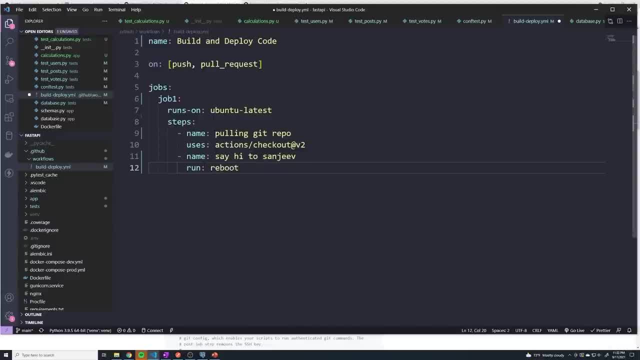 Or if you want to reload the machine. you know you could do a reboot. I'm not sure why you would do that. So all I'm just going to do is I'm going to just make it say echo, which is just going to echo out exactly what I type in here. 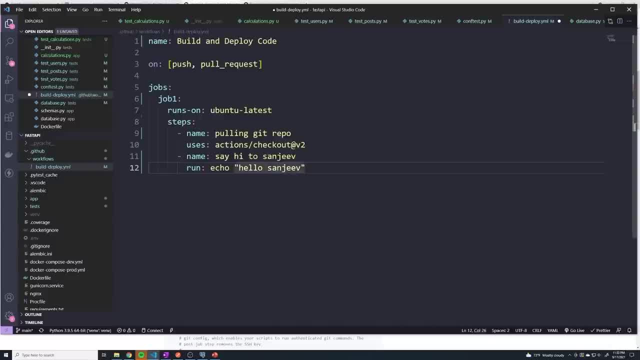 I'm going to say hello Sanjeev, And so it's just going to run this command on our Linux, And so this is a very simple example so far, but I think that's a good starting point so that we can actually understand what's happening. 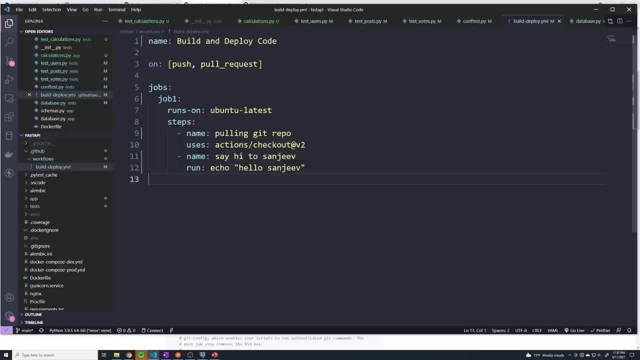 And what we want to do is we now want to actually push this changes to our Git repository. So let me open up my terminal, Make sure you do save all, And so once we push this, this will actually be part of our repository. 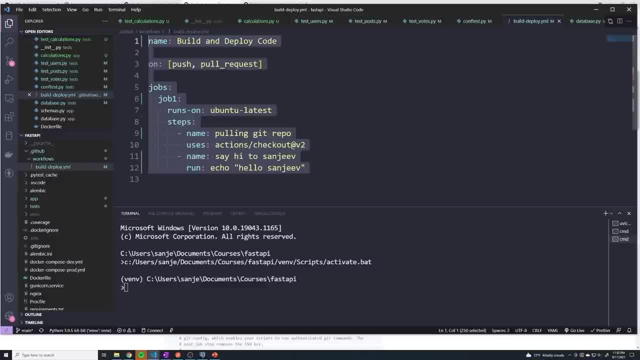 And it's going to actually trigger GitHub actions, to actually trigger this workflow, Because we said that on every push We should run this workflow. So I'll do a git add all, I'll do a git push. Sorry, git commit dash. m adding first GitHub action. 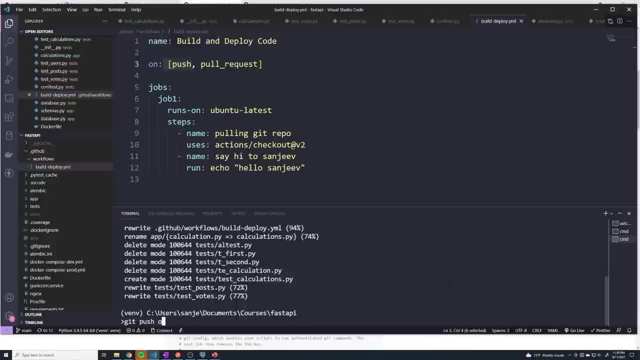 And then we'll do a git push And we can do an origin main if you want to be specific. All right, so it's been pushed, And so now, if we go to our GitHub repository, there's a actions tab right here. 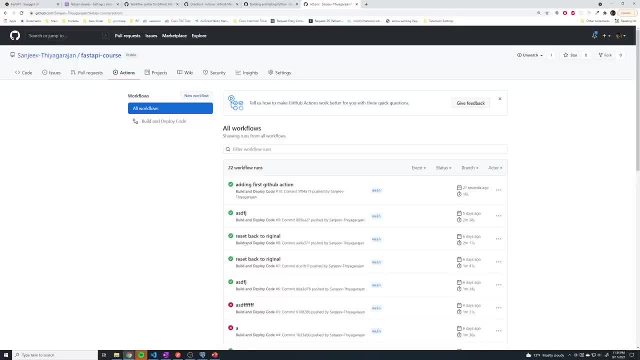 And so you'll see that I had a previous. I had a couple of other actions that ran because I was, you know, doing a dry run, but you'll see that the most recent one, which is the one we had, which is called adding first GitHub action. 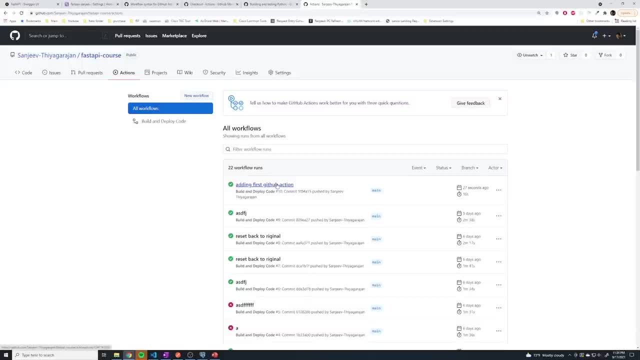 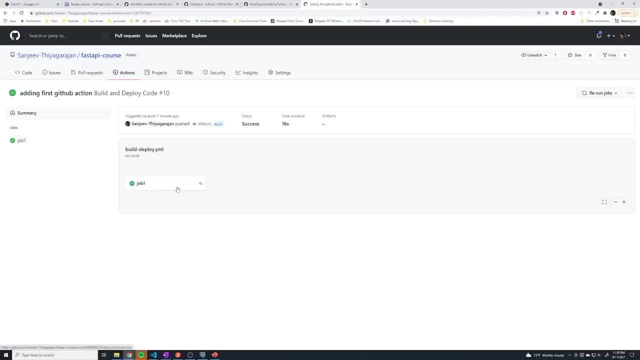 So this actually comes from the commit name and we could select this and we can see exactly what happened. So this gives us a little summary. We can see that we have one job called job one, and then we can see that the job ran, and it successfully ran and it took four seconds. 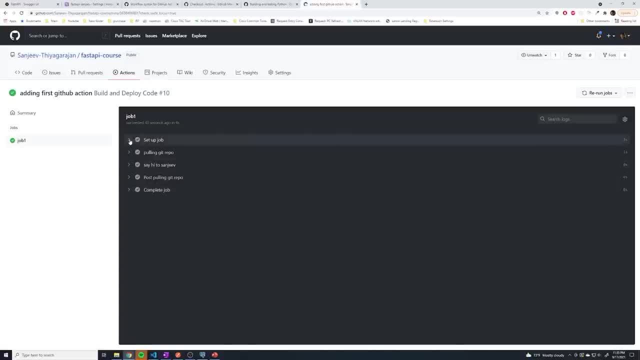 And if you click on the job, you'll see all of the steps. So The first thing is it sets up the job, and so you can see that it's creating a runner, which is once again just a virtual machine, and then it's going to provide us Ubuntu, because we specified that as our operating system. it's going to set up a virtual environment. 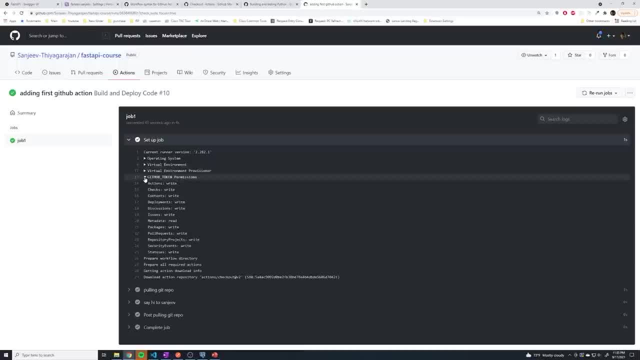 Don't worry too much about that. It's going to handle all of the GitHub permissions because it's all integrated with GitHub. Then we go down to the first action, which was pulling the Git repo, because we did say action slash checkout V2.. 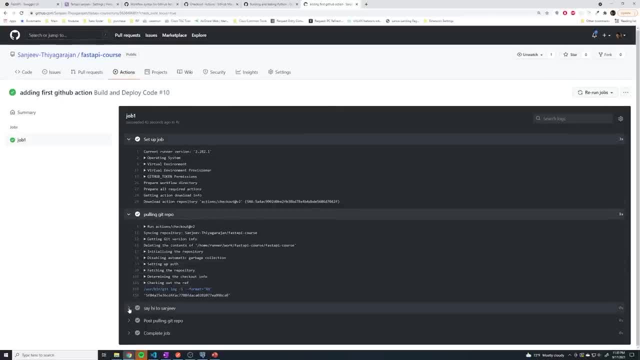 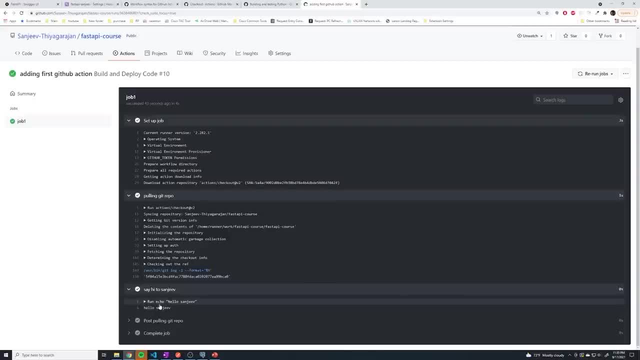 So then it's going to pull the GitHub repo and then we could see the second action- Sorry, the second action, which was say hi to Sanjeev. So all it's doing is just running this command on our Linux machine, that's just saying echo, hello Sanjeev. and then it just prints out: hello Sanjeev. 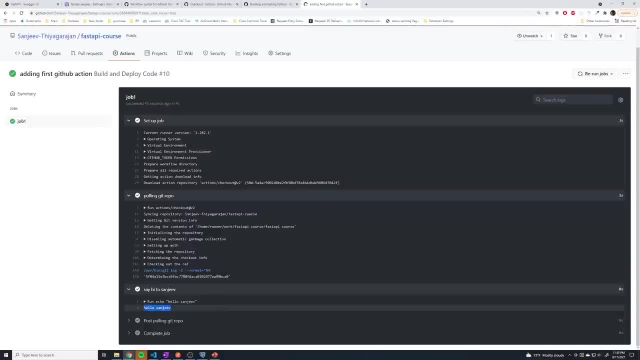 So this is all a CI CD pipeline is? It's just providing a bunch of instructions for a little machine on the Internet to run for us. Now, technically, the machine doesn't have to be on the Internet, It doesn't have to be hosted. 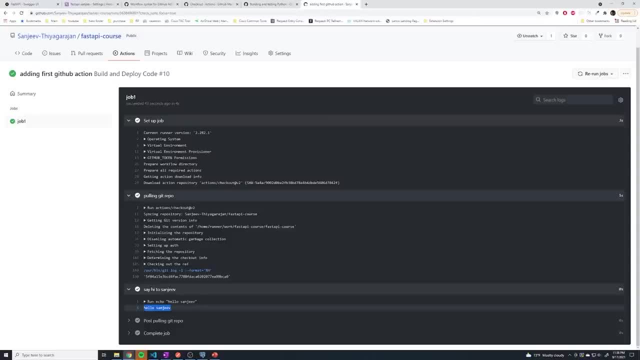 There's some CI CD tools that you host to yourselves on your, on your own machine or your own server, so that they actually handle running all of this. Because Even though GitHub actions is free, they only give you a certain number of build minutes for free and then after that they'll start charging for it. 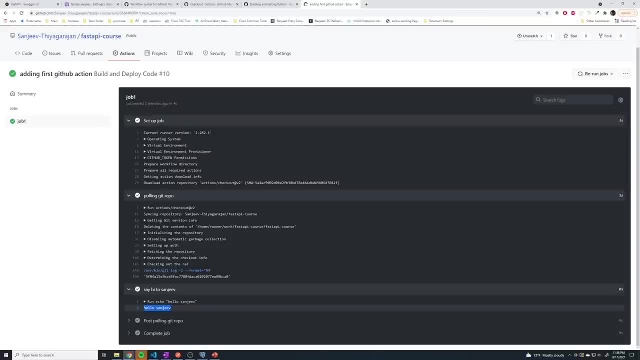 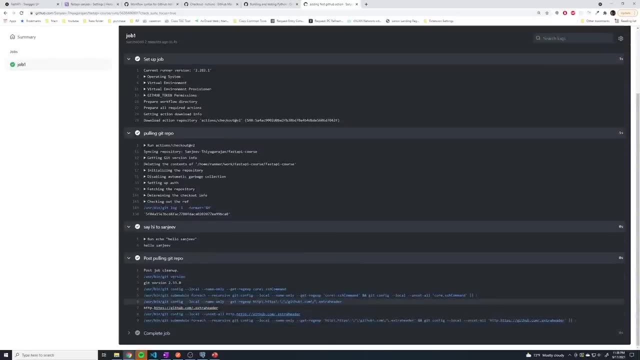 So, depending on how many times you build, it may actually be more cost effective to just set it up yourself. And then it looks like you know GitHub actions. there's a post pulling Git repo, so it's going to perform a few other like cleanup actions and then it's going to then clean up the job. 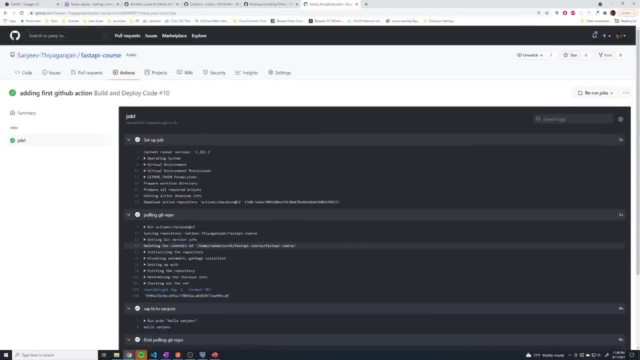 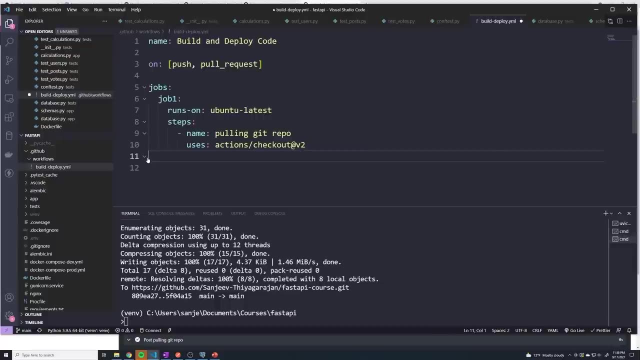 So we have successfully created our first simple example: CI, CD pipeline or GitHub actions workflow in this case. So let's take our GitHub actions to the next step And I'm going to actually remove this example. I just wanted to show you guys how to do that. 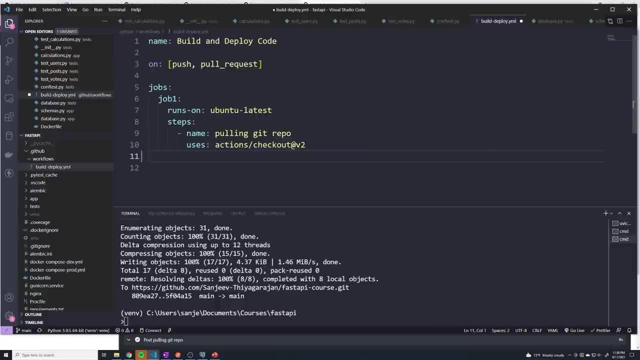 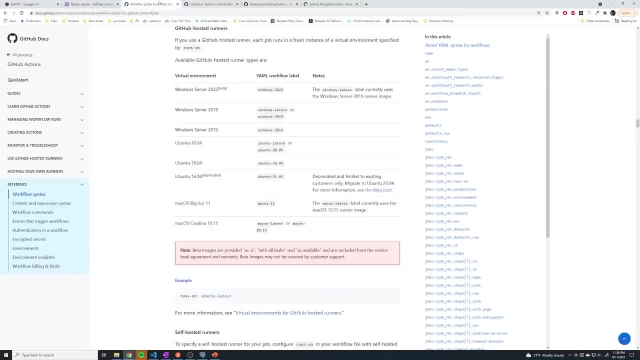 But after we pull our GitHub repo, the next thing that I want to do is I want to set up Python, And so to set up Python once again, we can go back to the marketplace, if I can find it, Because, you know, setting up Python seems like a very common task, so we can just search for Python. 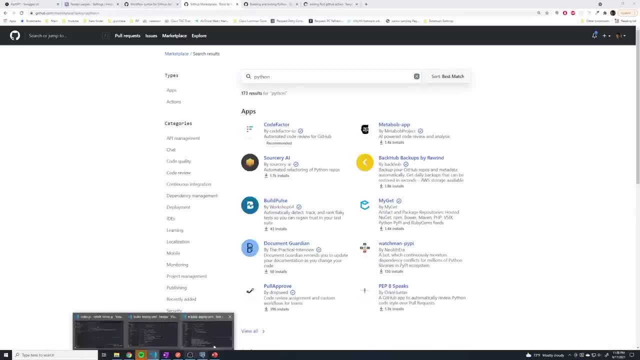 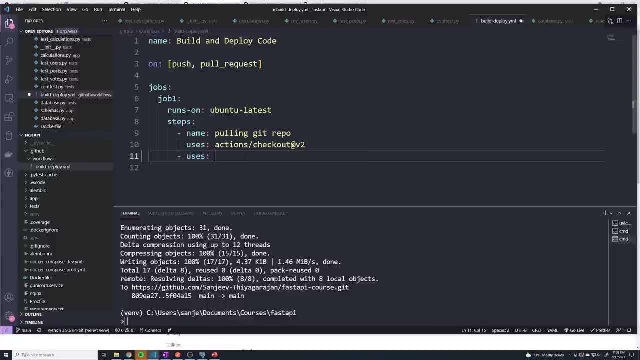 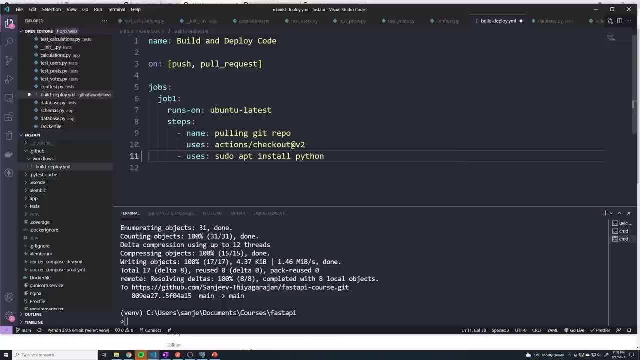 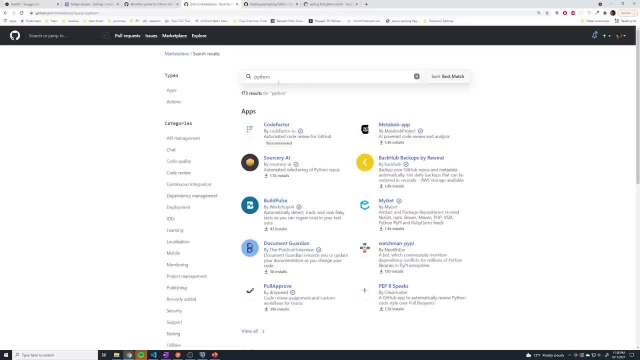 Right, We could 100% do that and that would 100% work. But because this is such a common task, there's already a prebuilt action, so we don't even have to do that, And I think I searched Python. 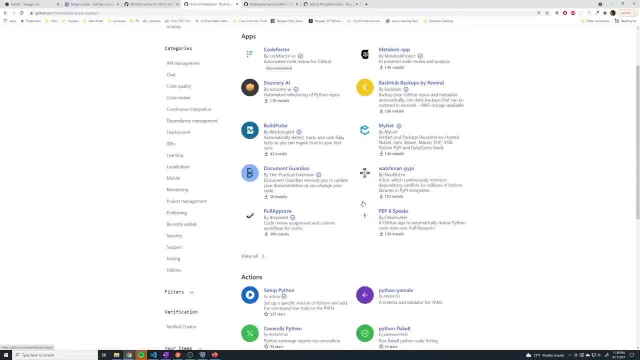 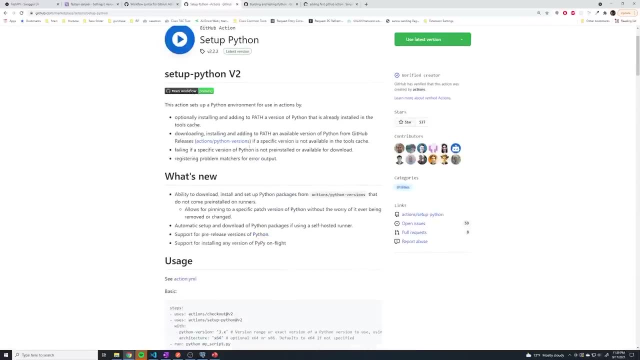 Did that work? It didn't look like it worked. Here we go, Set up Python down here. So this is going to be responsible for setting up and installing Python on our machine, and you'll see an example of how to do this. 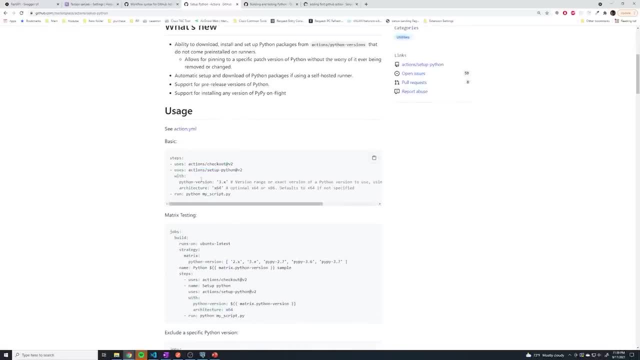 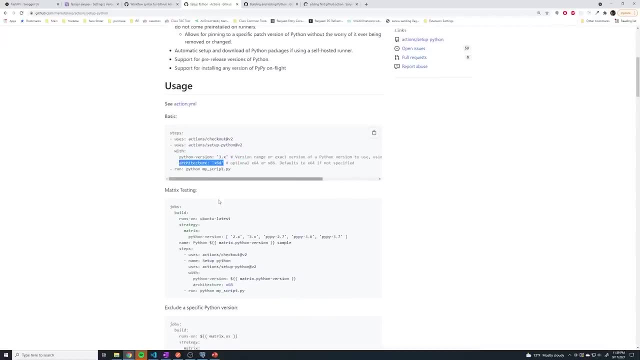 You just say: uses actions slash. set up Python at V2, and then you say with: and then you specify the version, and then you can also provide the architecture as well. And what's really cool about this is that, let's say, we wanted to test our code on multiple different versions of Python. 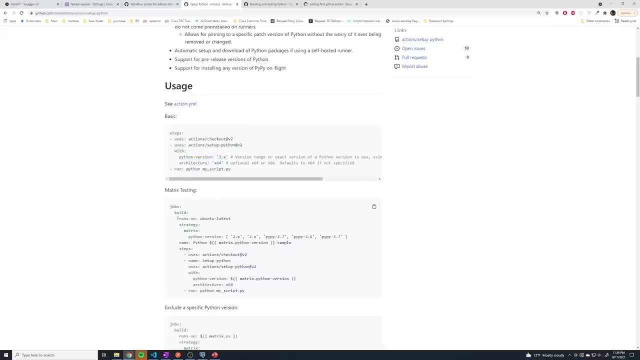 Well, we can go under the strategy section, So right under where it says runs on, we can do strategy, And then we can provide a version, And then we can provide a version, And then we can provide a matrix and then a list of versions. 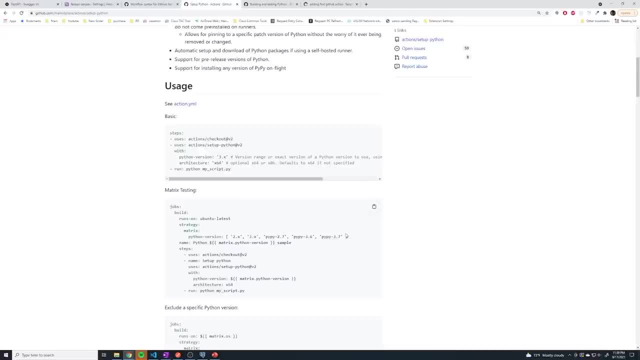 So if we wanted to test version 3.7, version 3.8,, 3.9,, 3.6, and make sure that our code works on all of them, we can then create this matrix here And then when we go to set up our Python right, we would say with and then for Python version, instead of providing one specific version we actually pass. 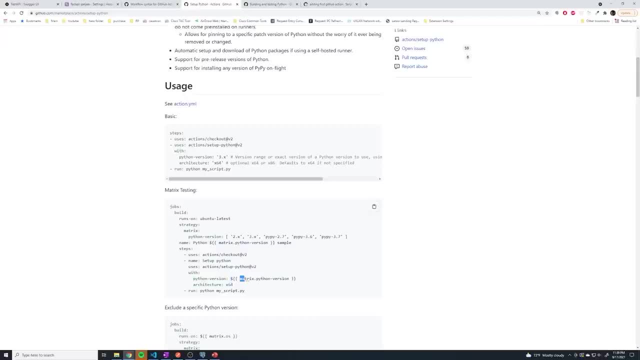 This is essentially a variable syntax in YAML, And then we just call matrix dot Python version, which is referencing this list right here, And so it'll just run our actions for all of these versions. It's just going to run it on all of these versions. 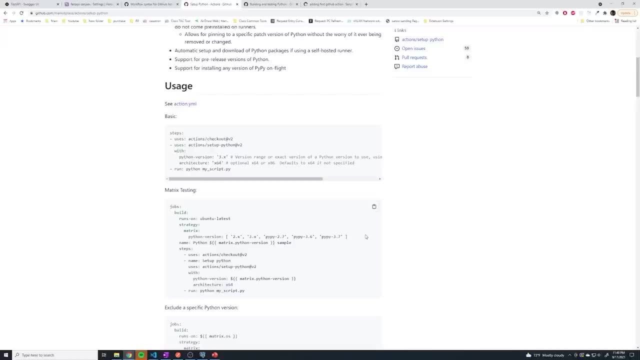 Okay, So let's do that of these versions, just to verify that everything works in all of the versions. But we're going to keep it simple. We're just going to do version 3.9.. If you want to play around with it, I definitely. 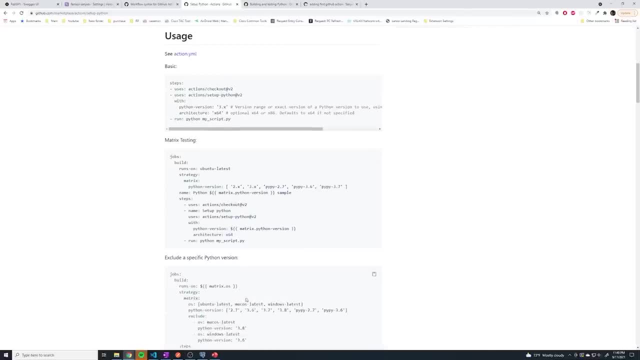 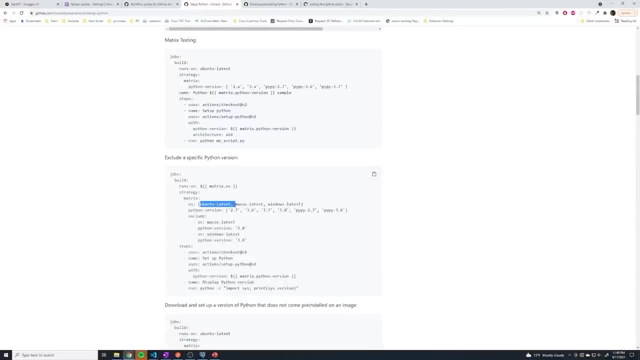 recommend you try testing this out, But for us it doesn't really matter. But keep in mind, it looks like you can even do the same thing for different operating systems. So if you want to test on Ubuntu, Mac and Windows, you can do the same thing as well. But like I said, we're going. 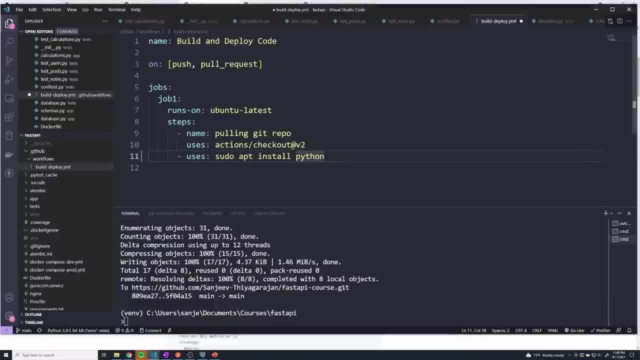 to keep things very simple- And I'm actually going to change this to name, give this a name. I'm going to say install Python version 3.9.. And then we'll say uses and then we'll call that action now. So we'll do action slash setup dash Python at v2.. And then we pass in with tab And. 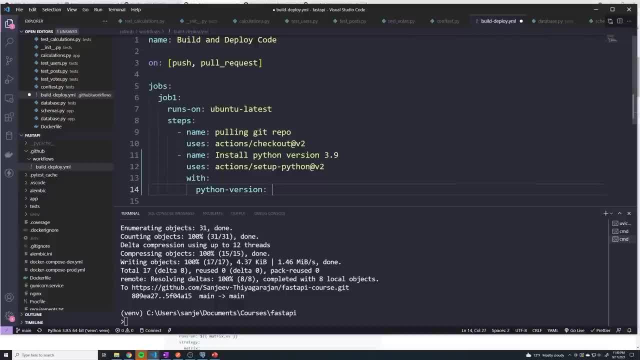 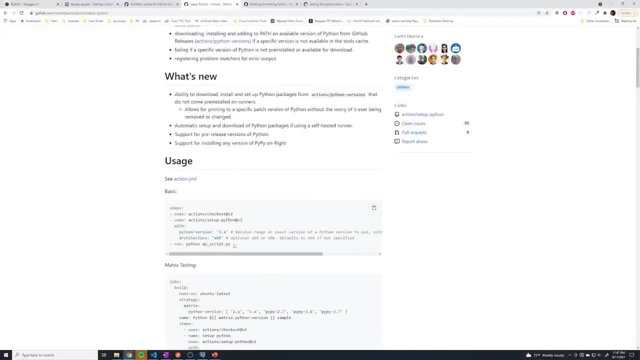 we'll say Python dash version, And we'll say 3.9.. And I think that's all we have to do. Let me see the example: Python version 3.9.. Yep, that's all. we can leave the architecture. I'm going to use the default. 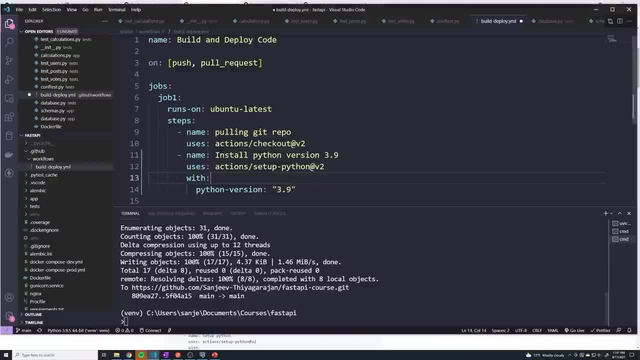 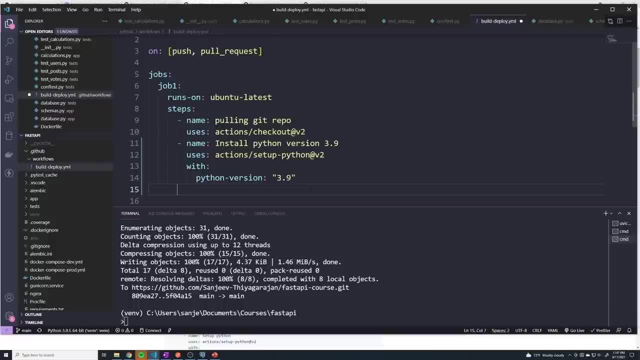 which looks like it defaults to x64.. So not a problem in our case. All right, and then, after installing Python, the next thing that I want to do is I want to upgrade pip, So I'll create a a description of update pip, And then we'll say uses Actually, instead of uses. 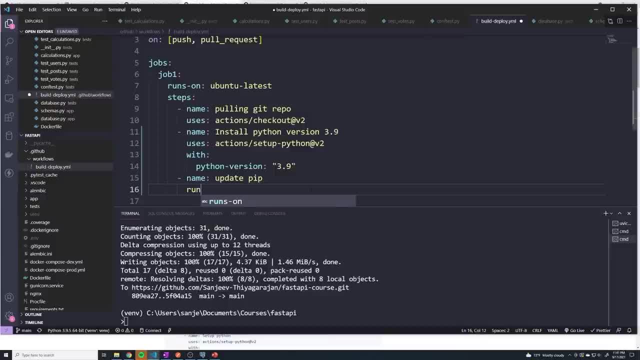 we're just going to run a command on the, the Linux shell, So we'll say run, And we just run: Python dash m pip, install dash dash, upgrade pip. So this is the command that you'd run on any Linux operating system or even on a Windows machine to upgrade pip. And then the next: 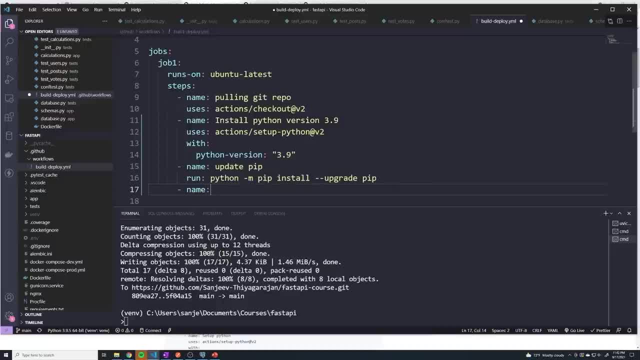 thing that I want to do is we're going to install all of our dependencies. So, since we pulled our git repo right with the actions checkout, we're going to have access to all of this code And we're going to have access to our 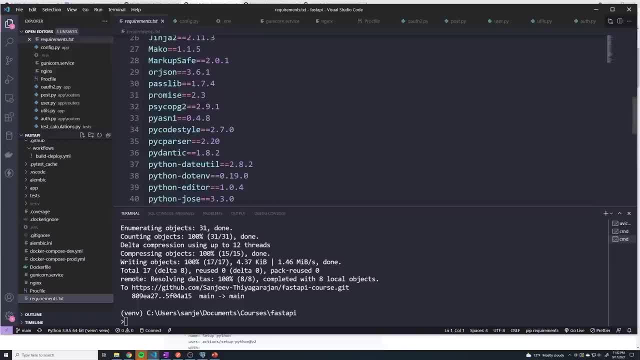 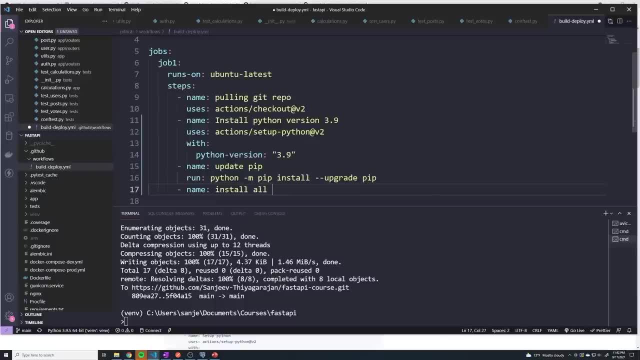 requirementstxt. So we have to make sure that we install all of these packages there as well. And so here I'll just say: this is installing all dependencies, And the command that we're going to run for this is going to be a, and you guys should know this. this is just pip install. 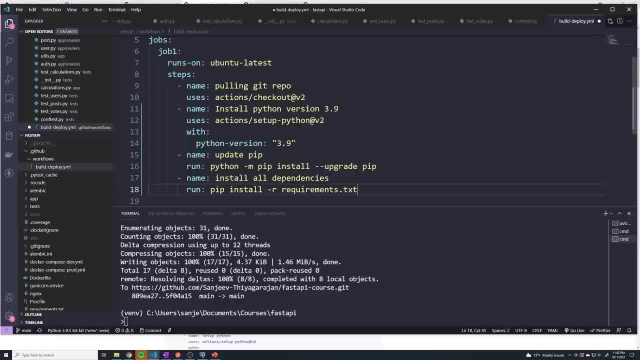 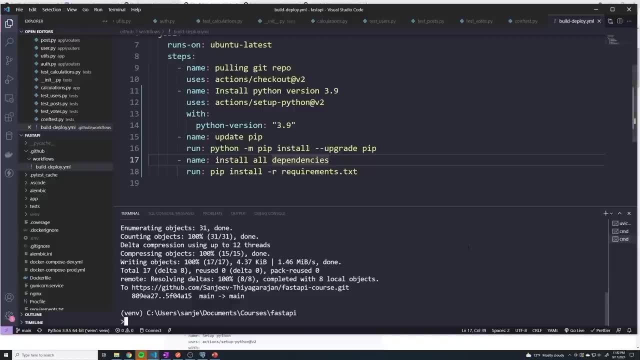 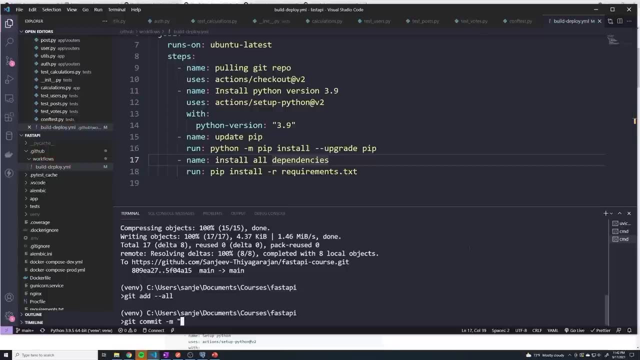 dash r requirements dot txt. Alright, so let's- I think this is a good starting point- Let's try committing our code again. I'll just do git: add dash dash. all. we'll do a git commit dash m added more steps. 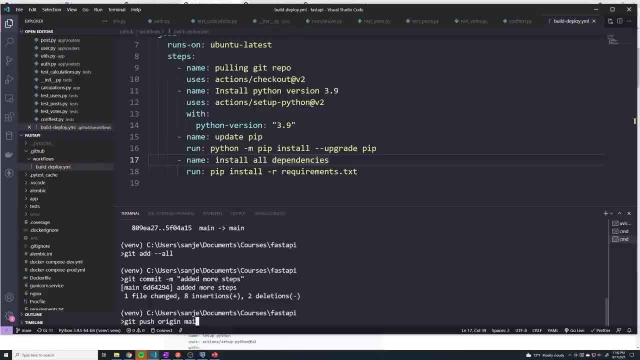 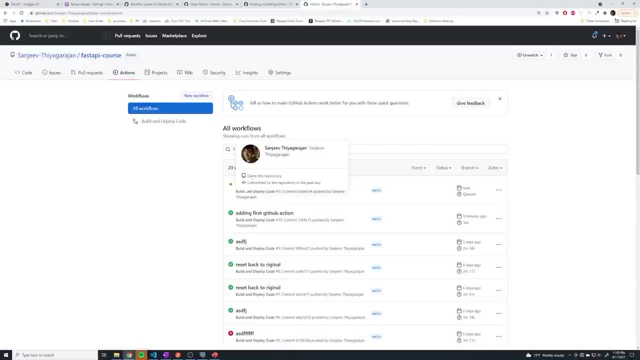 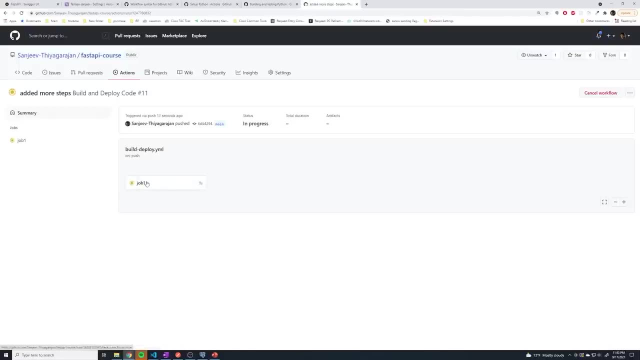 And then we'll do a git push origin main, All right, and then we'll go back to actions- Right, and we can see that our workflow is starting to run. That's why it's yellow And we can take a look at its current status. So it's still running, job one. 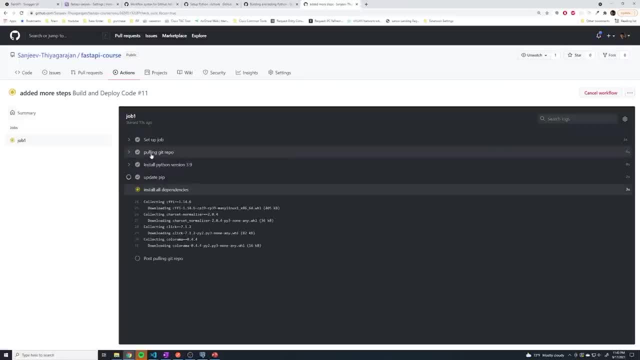 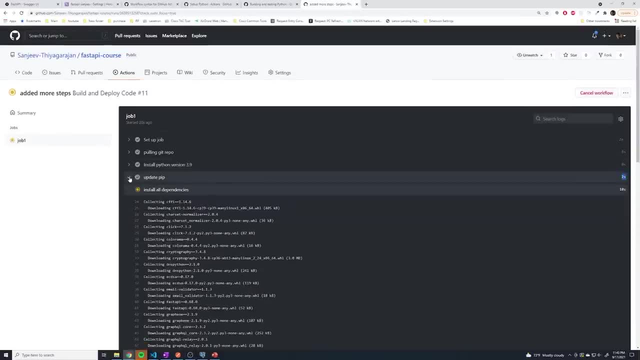 which is the name we gave it, And we can just kind of follow along. So it looks like it pulled our repo install- whoops, installed Python version 3.9.. It's then an updated pip and that's already completed, And now it's installing all the dependencies, So obviously installing all. 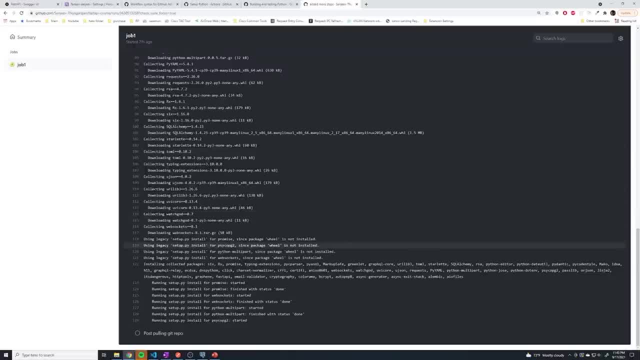 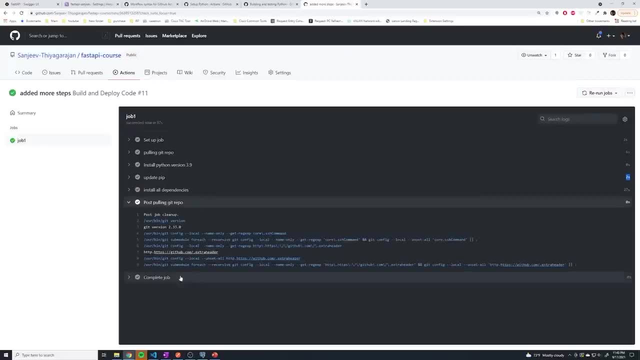 the dependencies takes a certain amount of time. that's probably gonna be the longest specific step in our GitHub workflow at this point. All right, and it looks like that ran And then it's essentially cleaning things up And then it's completed and we get the beautiful green checkmark So we can just close out of this go. 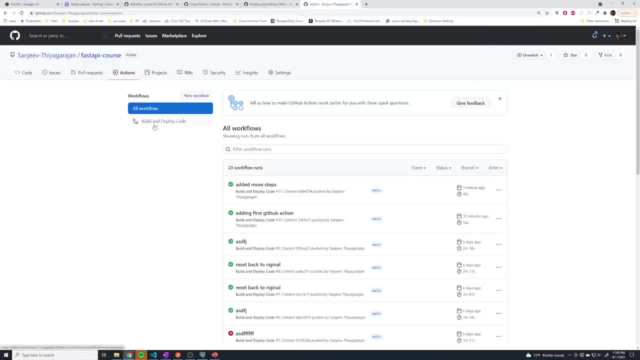 back And you can even see the list of all of our workflows- that GitHub actions is detected. So we have built in deploy code. So that's the only workflow that we have. But keep in mind I can create essentially as many different YAML files inside this workflow folders. 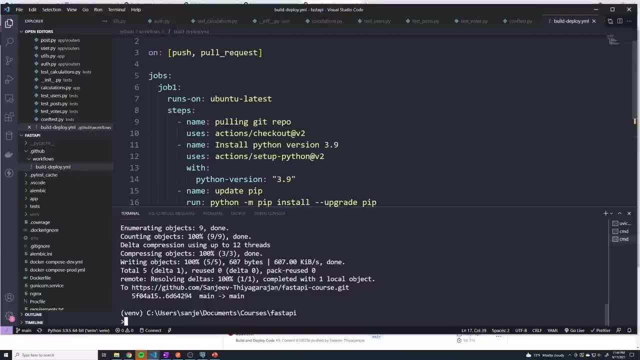 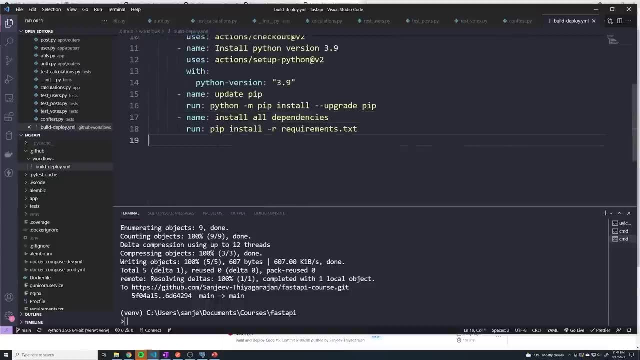 to have a different workflow, So I might have one specific set of. I might have a workflow specifically for one branch and a completely separate workflow for another branch. It just gives you a lot of customizability, But we're just going to have one workflow that works across all of our branches. Now the next thing that I want to do is I want to 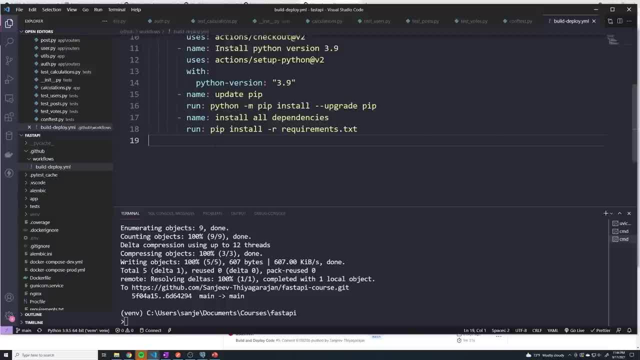 run pytest. So to run pytest right, it's a pretty simple process. So let me set up the name. first I will say whoops, test with pytest. And then we'll say run. All right, and I need to run two commands. So if you ever want to provide a list of commands to run, 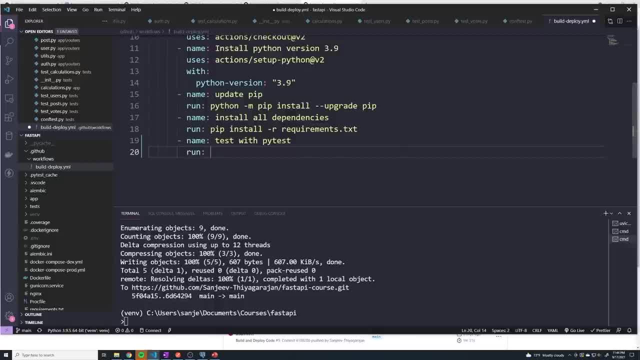 instead of having to create multiple different steps, I can do a pipe, go down the line and just provide the list of commands. So we'll do pip, install pytest. And then we can go down the line and provide the second command. So then we just run pytest And you can. you know. 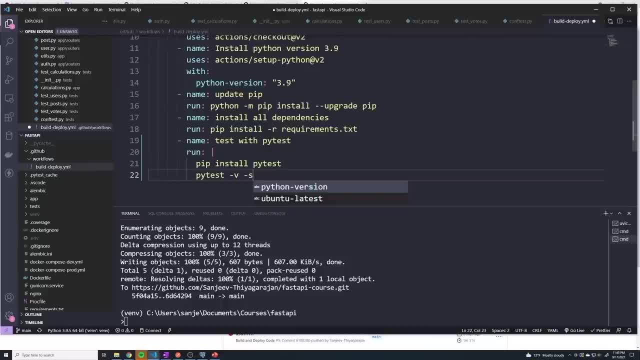 pass in whatever flags if you want- the dash v and the dash s- But I'm going to keep it simple And we're just going to keep it blank. for now, Let's save this And I'm going to then do the same thing. We'll do a git: add dash, dash, all. 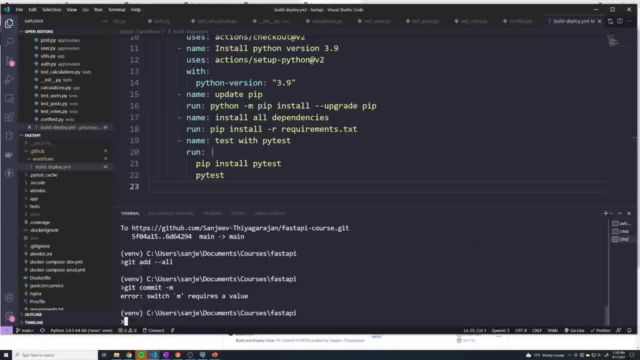 we'll do a git commit dash m And I'll say added pytest step. And then we'll do a git push origin main again. And so, from from a learning perspective, right, this is kind of a slow process because we have to push all of our changes And then now we have to wait for this. 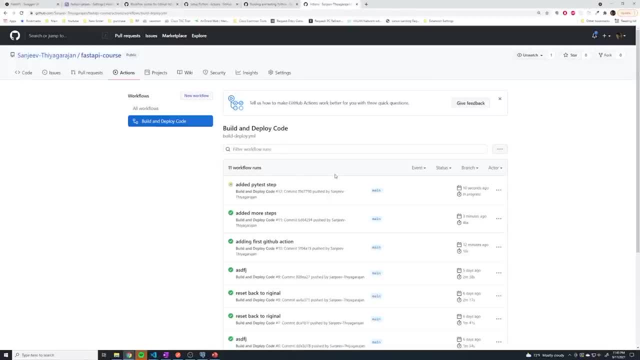 whole thing to run, But I'll wait for it. Once you understand how all of this works and how easy it is to set up, you won't have to keep doing this every single time or every single project. you can just essentially copy and paste most of your workflow. 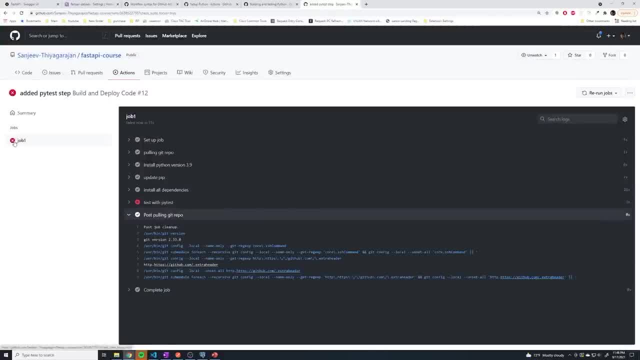 Alright, so it looks like it's completed and we get a red x, So it looks like something broke And that's to be expected And it's going to highlight what specific test failed or, sorry, what specific step failed, but we can see that it was the running pytest. 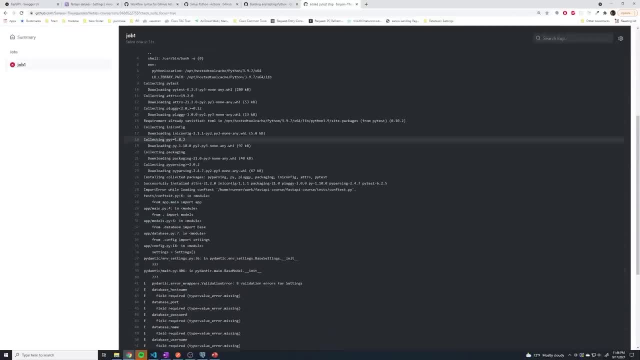 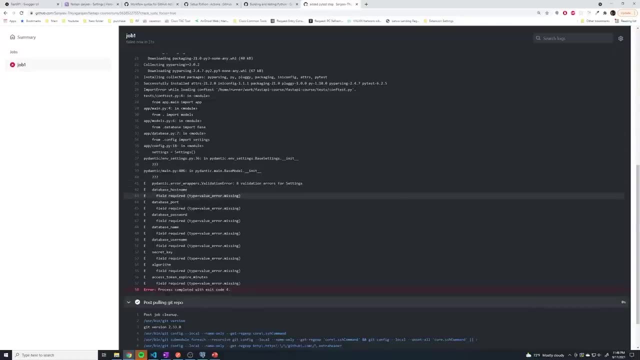 So if I just open this up a bit and then expand it, we can take a look at what the error was. So it looks like it installed pytest And that seems to have worked fine, And then down here you can see that there's a couple of validation errors. 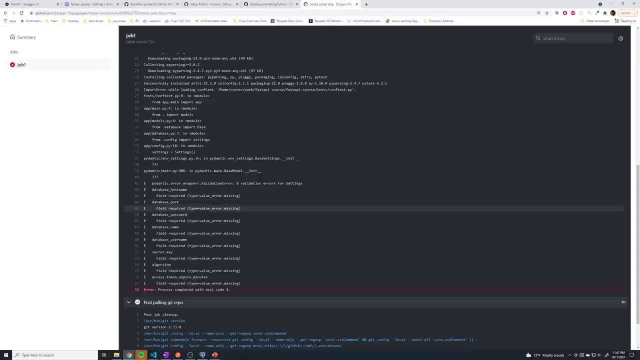 And so it says that you know we didn't provide a database hostname port. So it looks like there's the issues with environment variables. And that makes sense, because this is a brand new computer that we haven't touched, So none of the environment variables have been set up, So obviously it has no environment variables. 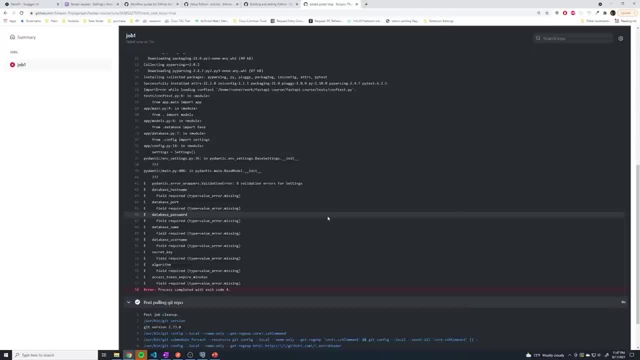 and then our pydantic validation of environment variables should have failed- and it didn't Absolutely fail. So this is all to be expected, And so in the next video, we'll figure out how we can set environment variables in our workflows so that we can provide the information for reaching 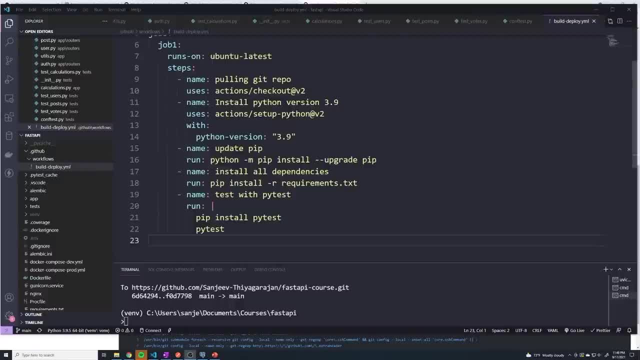 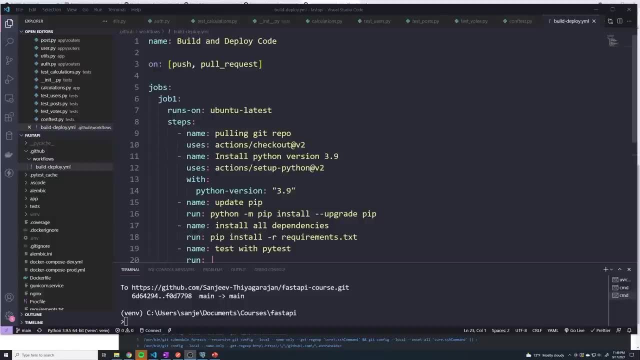 our specific database. So there's a couple of different ways that we can set up environment variables And there's a couple of different places where we can define them. So I'm going to show you a job: how to set a job specific environment variable. That means this is an. 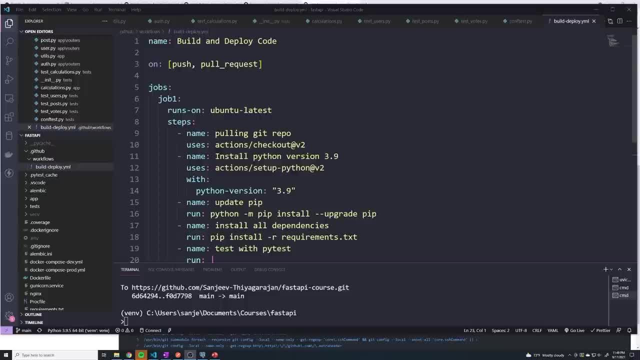 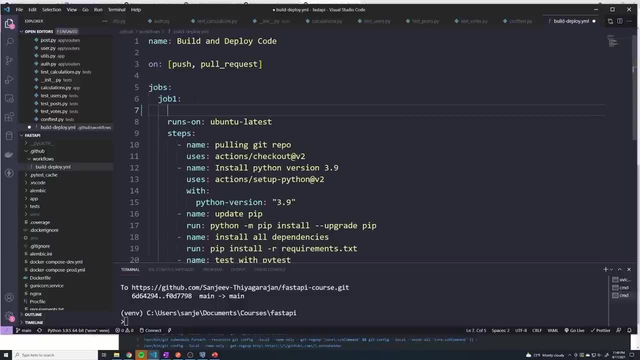 environment variable that will only be accessible from within one job. So in this case, our job that we've been working on is called job one, And so if you want to set an environment variable, you just set it right here. So we say ENV. 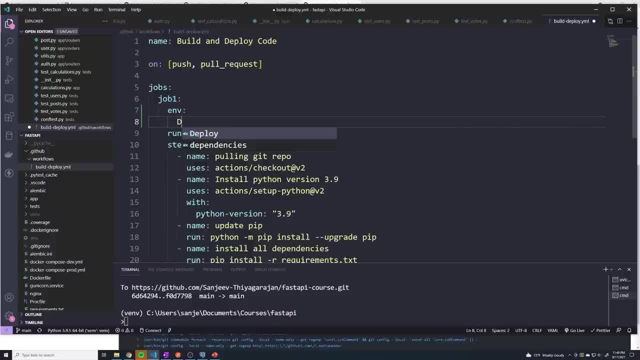 And then you provide all of your environment variables. So in this case, let's say we want database hostname And in this case it's going to be localhost. We've now successfully sent, set up one environment variable and I'm just going to copy and paste all the others. 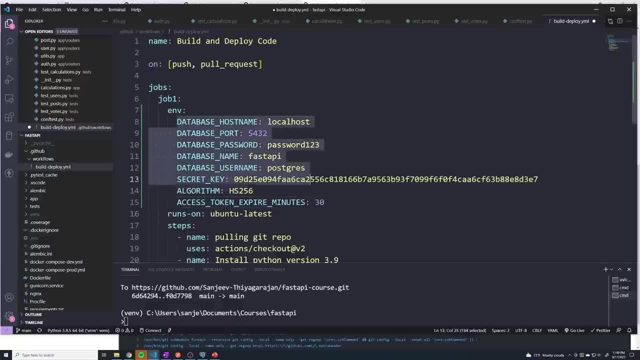 That will set up a behind the scenes initial variable, which are? are those controlled? I'm just saying this: All those control wiele Morning. and so now we've defined all of our environment variables in this case. Now I'm going to go ahead here and prove that we're success, And I don't know if you've seen, 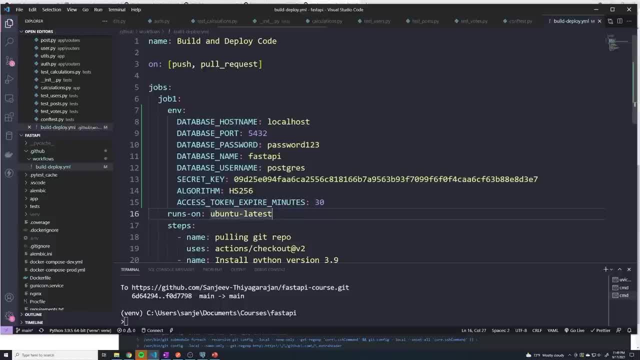 a pap, just basically a little bit of yourself again. That should fix the issue, But I want to show you guys what other environment variables that we have as well, And if you want to know where I'm kind of getting all this information. like I said, 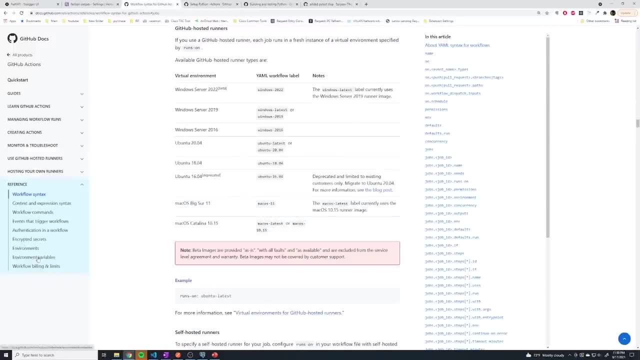 we have the documentation, and there should be a section for environment variables here, And so I think we should see the same thing, right? Yep, we see the same thing. So if you wanted to see my recentこちら eating a picture in the camp, 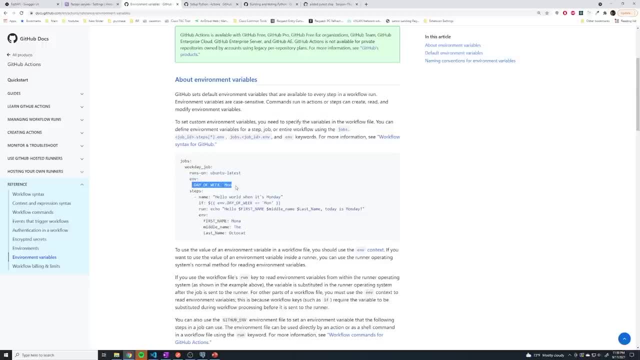 then how would that do for me? oh well, But finally, we're looking at dagen, smoar and V under the specific job, And you just provide the list of all of your environment variables And then there's some built in ones. So these are default environment variables that get set for. 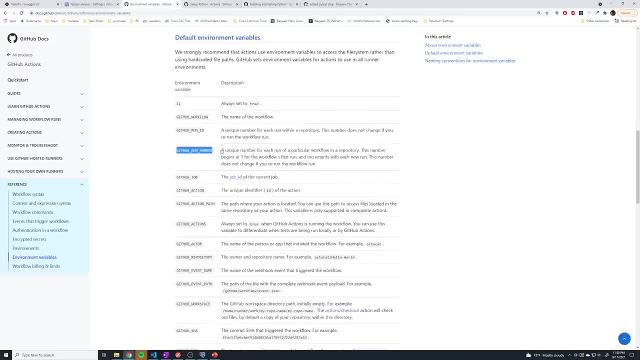 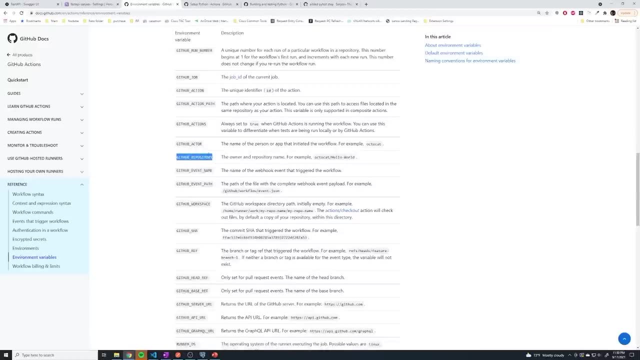 you. So here you can see what's the run number, what's the GitHub job, what's the action path. we can even see what's a repository. So if you want to get the name of your repository, you can reference this specific environment variable, but we don't need to do any of that. 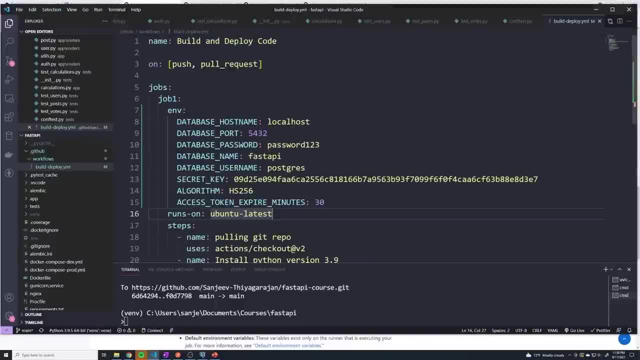 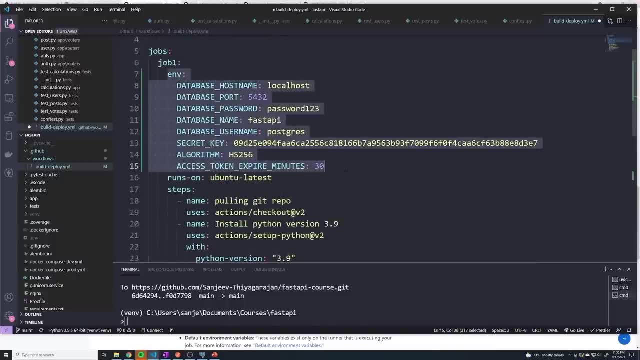 But what I do want to show you is: you know, if I had gone in and then created a second job called job two, right, this environment variable that we define here is not available because this is defined under job one. So if you want to have a environment variable that's shared across all of 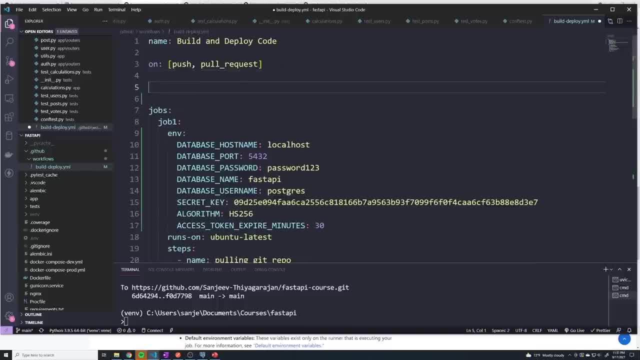 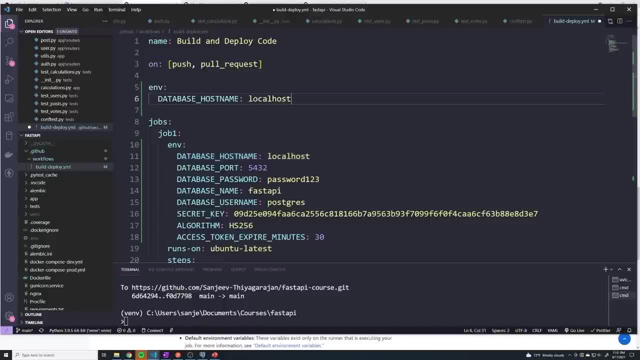 your jobs. I can specify an environment variable here. I can say ENV, And then I just provide my environment variable. So I can just copy this one as an example And we can provide this. So then database hostname is going to be available for job one and job two, But for now we're just going to remove that because we don't. 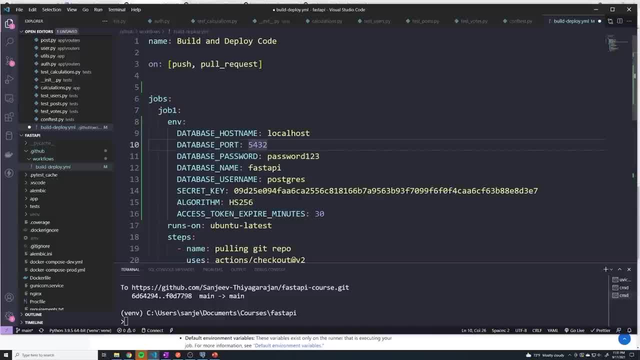 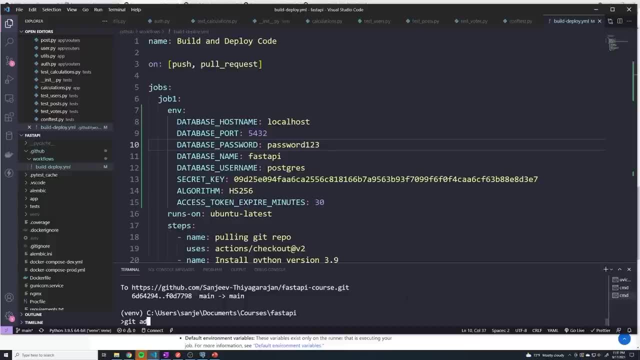 really need it. We don't really need that right now And I'm going to keep everything as default in this case, And we're going to check this into git. So I'm going to do a git add dash, dash, all. do a git commit dash, m, added ENV variables And we'll do a git push origin main. Okay, and then 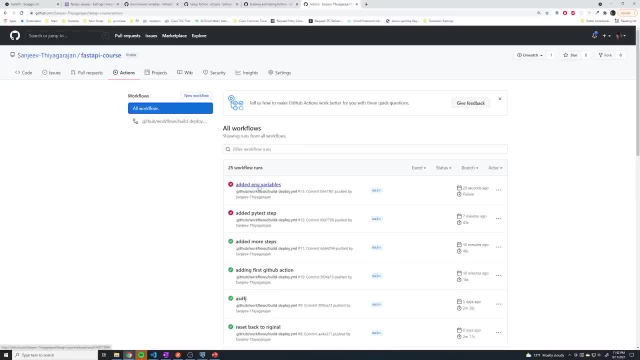 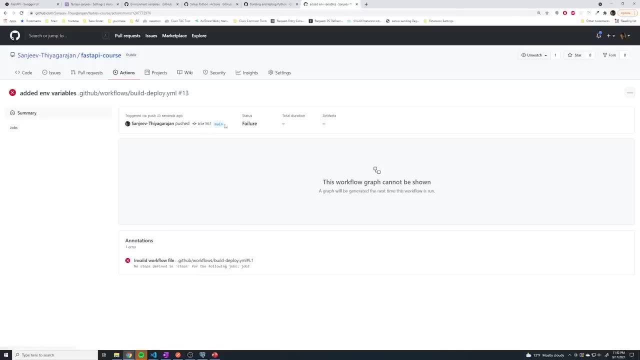 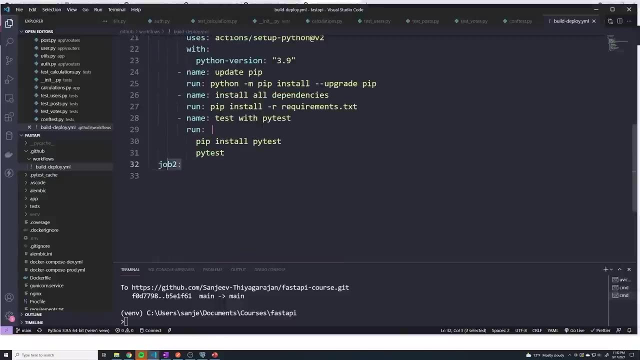 back to our actions page. If I see the added environment variable section, we can see that failed. Once again, this is going to be expected, So if we go under hope, it looks like there's a weird failure. no steps defined. Okay, so we got an error because I accidentally left job two, So it doesn't like it. 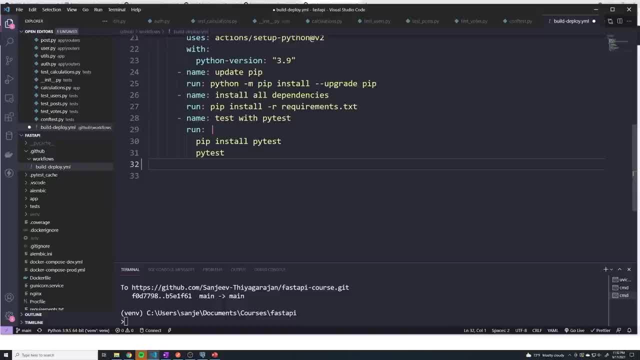 the fact that I have jobs, two with no steps. So we're going to save this again And we're going to do another commit, And I'll just call this committing again, because I'm getting lazy. Let's open up little orthalie, All right, and 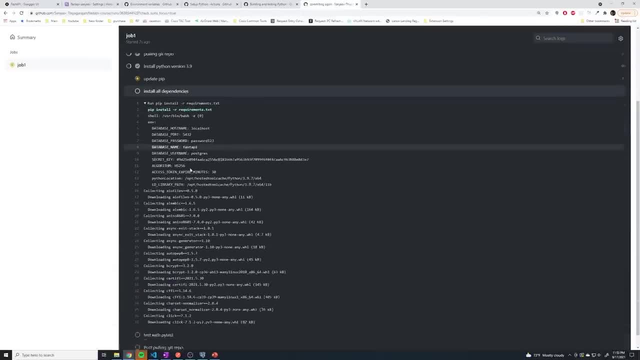 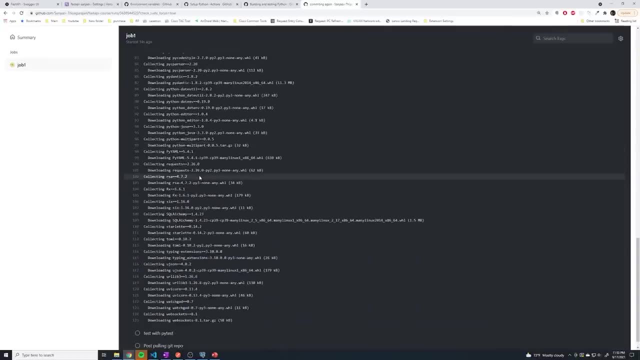 let's just make sure that we've kicked this off Alright. so it looks like you kicked it off and there's no like major show stopping errors at the beginning. But we should still see this fail, And that's to be expected. But just want to make sure that we no longer have issues with 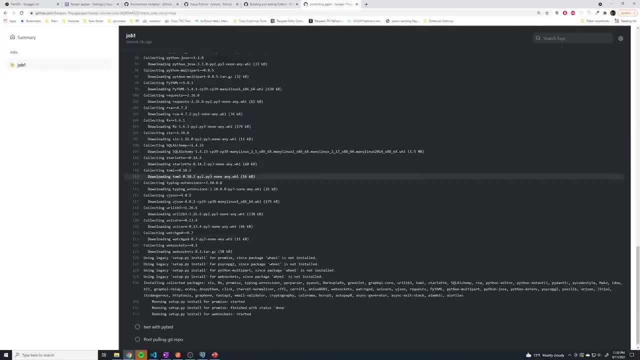 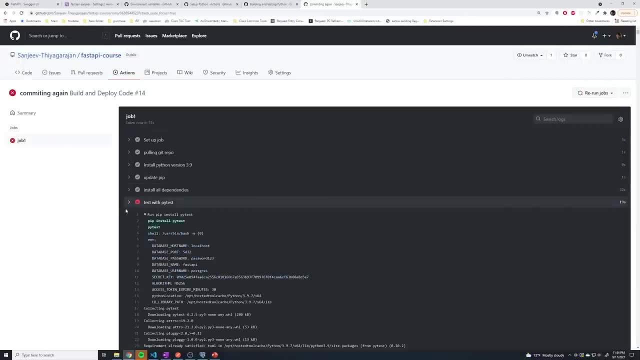 environment variables And I want to make sure that the very variables that we set did successfully get applied to our runner. Okay, guys. so So there's a whole bunch of errors, And that's to be expected And that's okay, But we can see that. 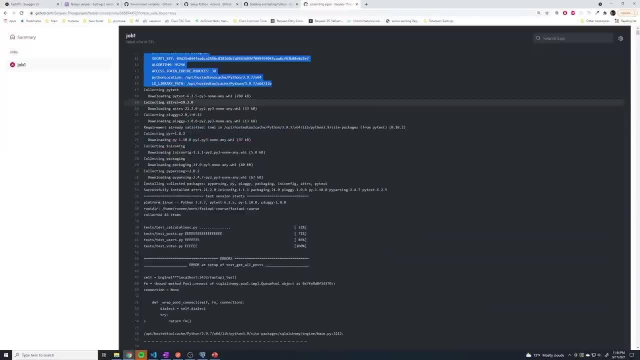 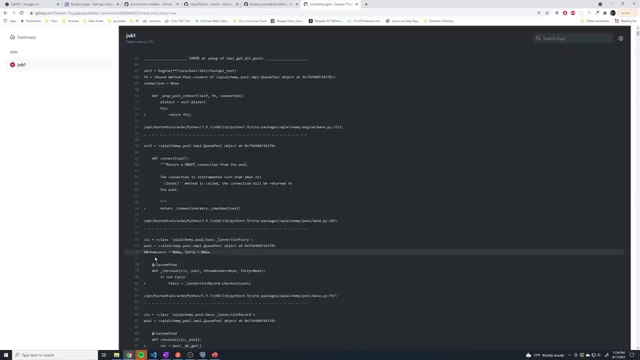 it did process all of our environment variables, So that's great. So we did fix that issue. But you'll notice that you know, when we're running our test we get a whole bunch of errors And then eventually you'll see a whole bunch of SQL alchemy errors And the reason. we see a whole 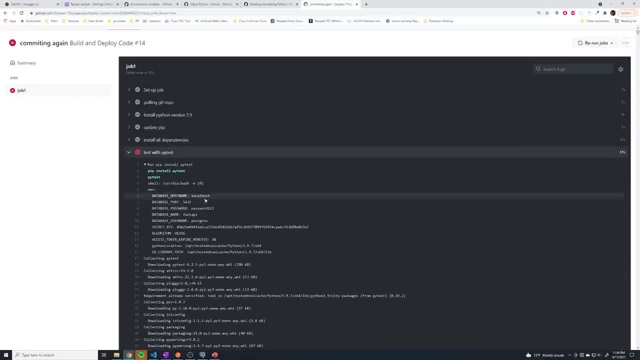 bunch of SQL alchemy errors is because if you look at the environment variables, we're pointing to local host for our database. there's no database on this runner. this is a brand new computer, that why would there be a database installed? So we do eventually have to set up a database for testing. 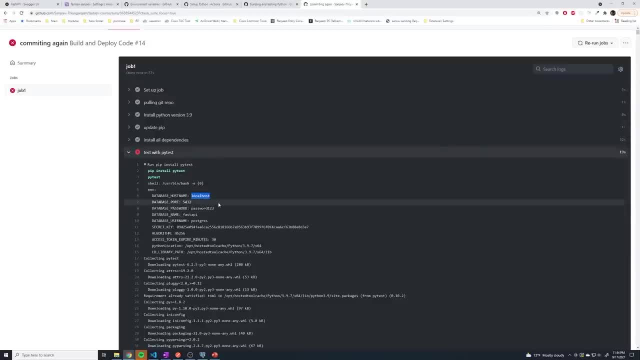 on the runner itself, or we would have to point it to a remote database. whether that's hosted on Heroku or AWS, it doesn't matter. But you know, for testing purposes in your CI CD pipeline, I'd rather create one on our runner that we can just quickly spin up for testing. 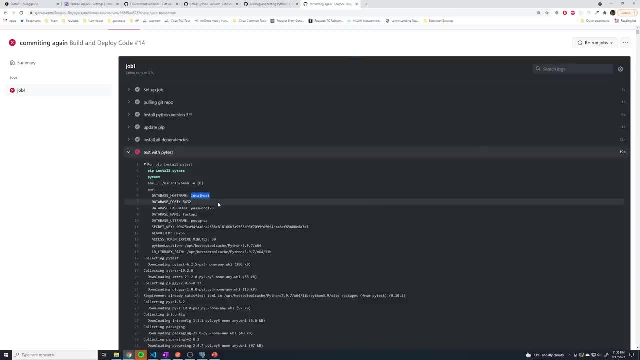 So, once again, I just wanted to point out how to set up environment variables. The one thing I don't like- and I want to make sure I want to teach you guys- is that in this case, we're hard coding these values. So we're going to set up environment variables and we're going to set up 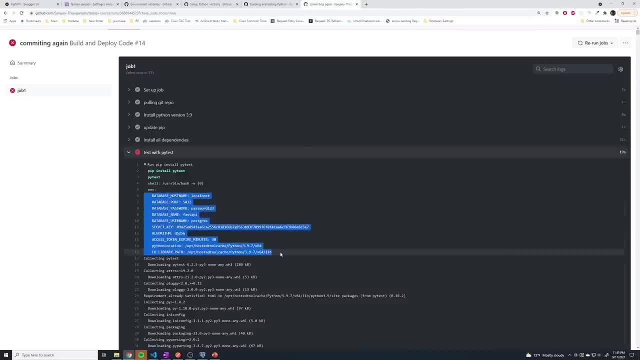 these values in here, And so this is all stored in our repository. anyone can have access to it. This is our test database, So it's not a big deal, But I do want to show you how we can, how we can, store these as secrets so that the runner has access to them but no one else can. 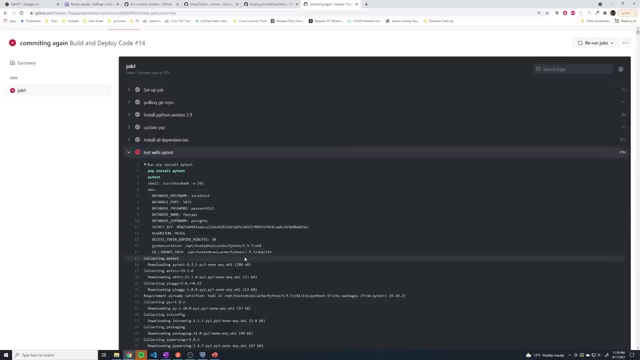 see them, because storing it in here could potentially cause issues. You know, if you didn't want this, these, these, the password and the username for your test database- to get out, In my case I don't really care. But you know it is important for you guys on to understand how to actually do that. 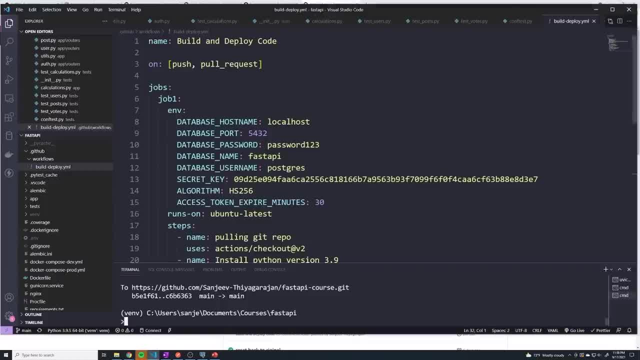 So, as I mentioned in the last video, our environment variables are hard coded into our workflow. So, technically, when we check this into get anyone can see it- which may or may not be a problem- But if it is a problem- I'm gonna show you guys how we can work with GitHub secrets. So 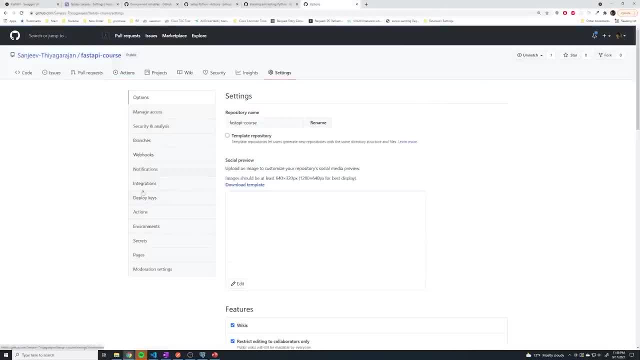 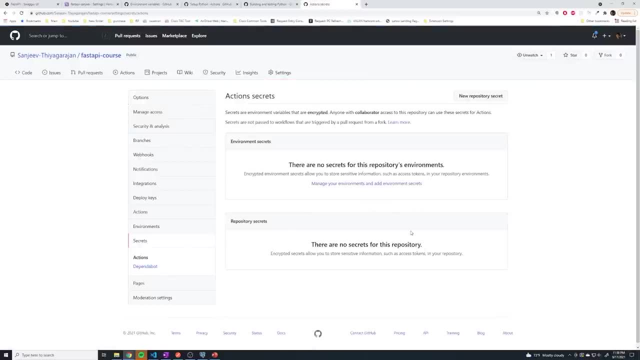 if we go to our GitHub page and go to settings, here there's a section called secrets, So we can define secrets that we can use and access in our workflows, And so this is a repository secret. That means it's globally accessible across the entire repository. 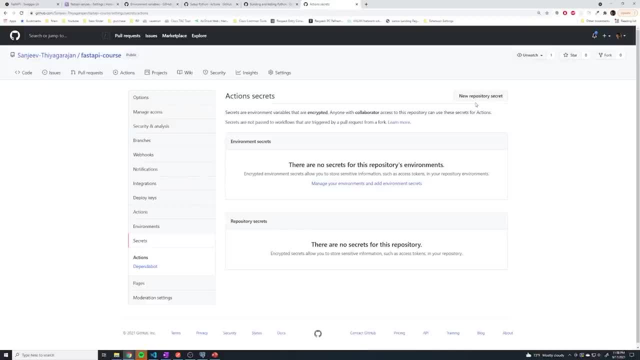 across all branches. There's no, you know, any kind of environments or anything like that. So we'll select new repository secret, And here we just give it a name. So if you take a look at our environment variables, I figured, since that's what it's going to represent, we might as well use the 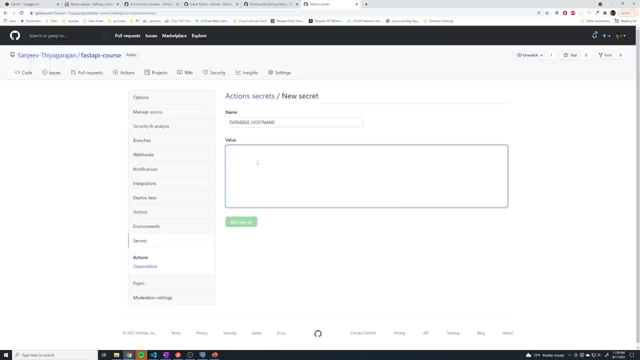 same one. So I'll say database, host name in this case, and then just give it a value, So local host. that's it right. It's just a key value pair. we do add secret And then you'll see it's stored in. 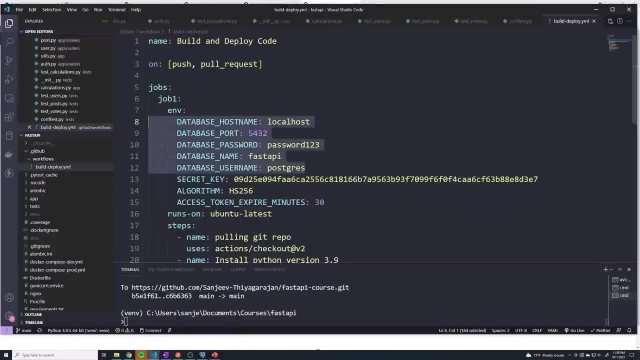 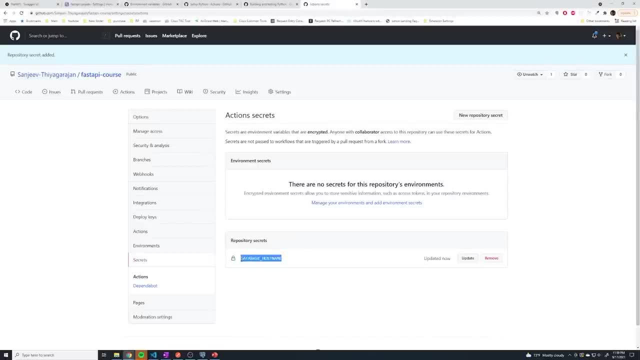 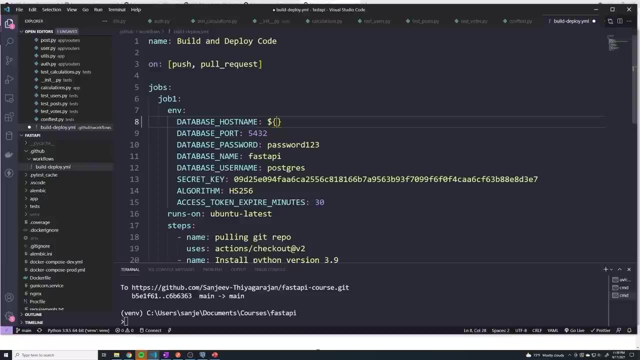 here. And so now in our code, if we want to reference the, this secret, which I happen to call database host name, we just copy the name of the secret. And then what we do is we use a dollar curly brace, curly brace, so two sets of curly braces, And we say: secrets dot and then the name. 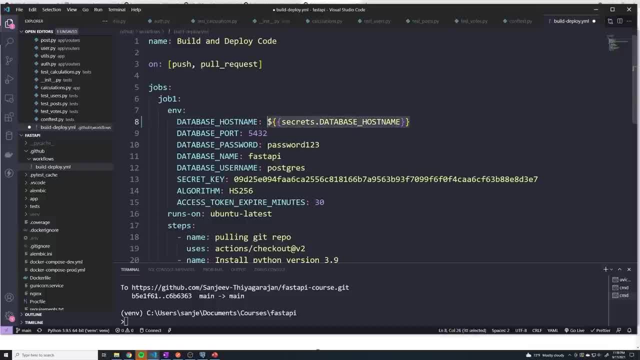 of the secret. So this will allow the runner to access the secret from our GitHub repo, so that our our flow code doesn't actually expose all of this information, And so this is what you want to do for your passwords and things like that, especially when 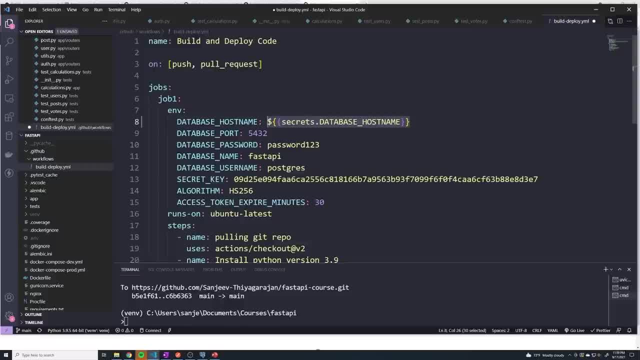 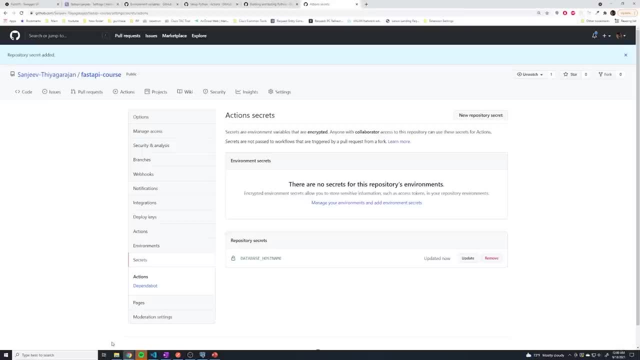 it comes to storing the information for connecting to your production database, which we will do in one of the later lessons. But before we proceed any further, I want to actually show you another option. So I'm actually going to remove this repository secret in this case, which is once. 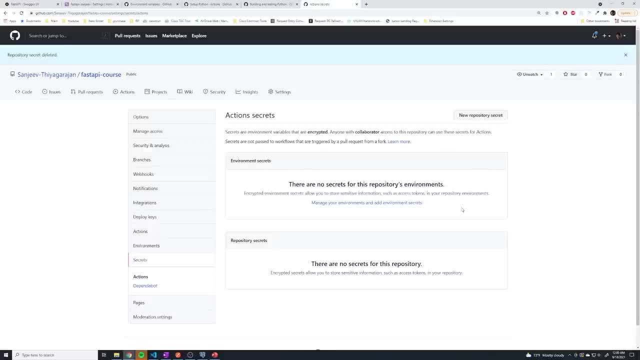 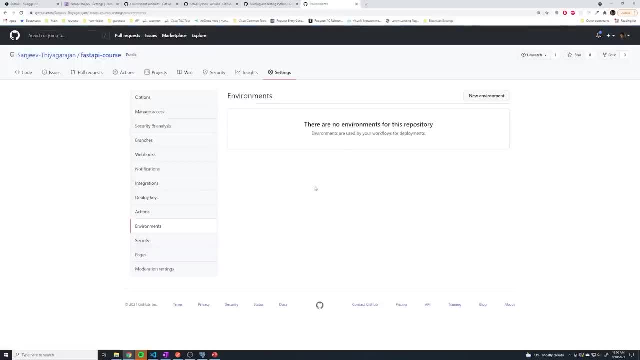 again a global secret that our entire repo can access. Instead, what I like to do is I like to set up environments, So you can set up a whole bunch of secrets that are available, depending on what the environment is. I can create one for testing, one for development, one for production. it gives us a lot of flexibility. So I'm going to create a new environment. I'm going to call this testing. 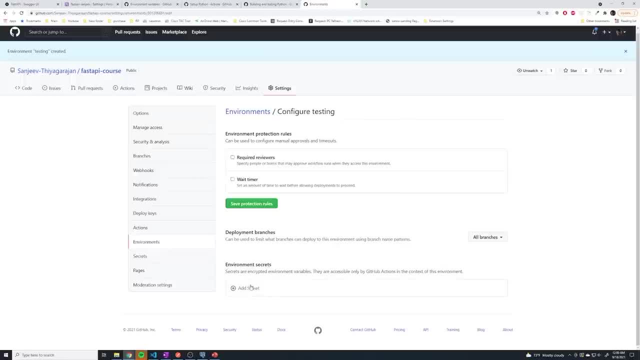 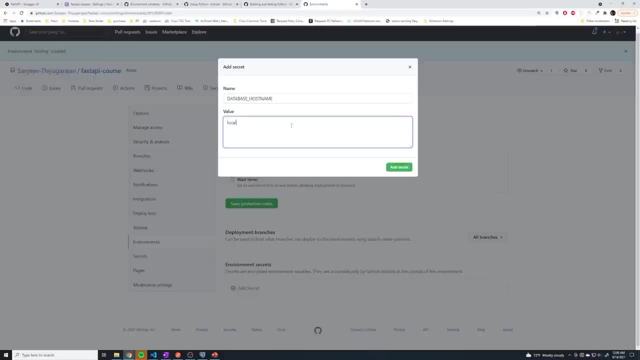 And within the environment. we're right, we're under the testing environment. we can add a secret here, And so we're gonna do the same. I'm gonna call a database host name and in this case we'll say localhost. we'll add the secret. 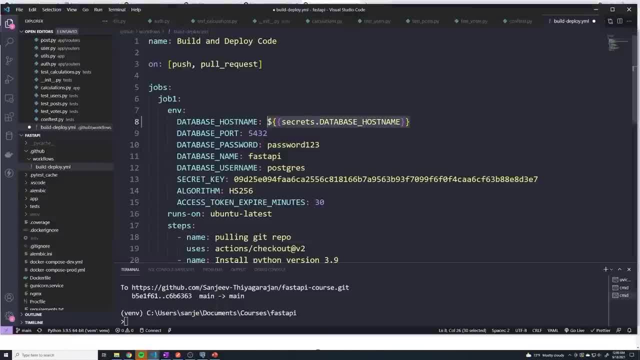 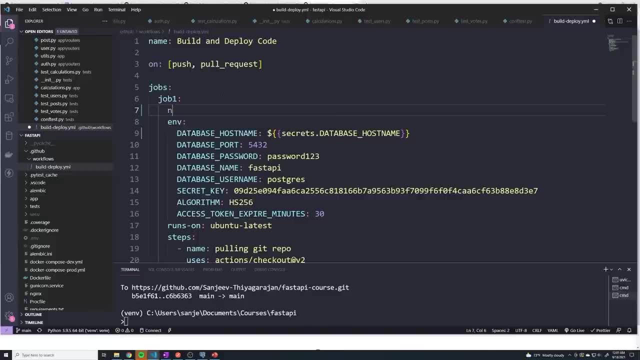 And we can provide as many secrets as we want. And then what we can do is, in our job, we can specify what the environment is for the job. So I can say, and oops, environment. And then we provide the name which is going to be. 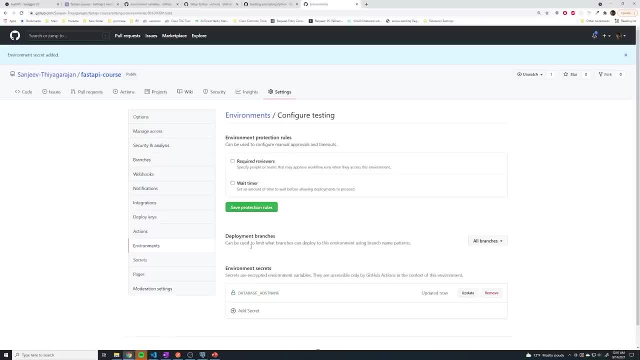 testing. right, This is going to match up with whatever name we gave here, So I called it testing, So we give this the name testing, and it's going to have access to all of the environment variables that we defined here And the way to access them. 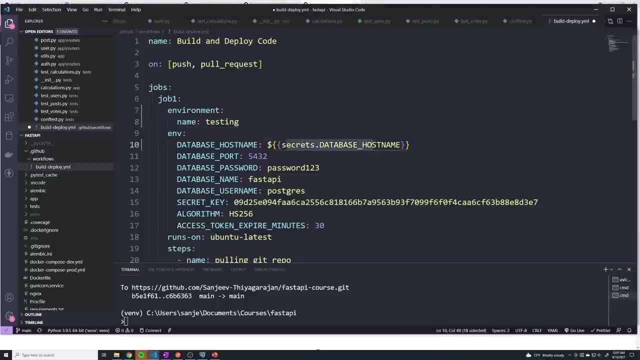 is exactly the same way. you just do dollar two, curly braces, secrets and then the name of the environment variable. Now, if there's an overlap with the name of your environment variables, when it comes to the ones that you set in your environment as well as the one you set globally- 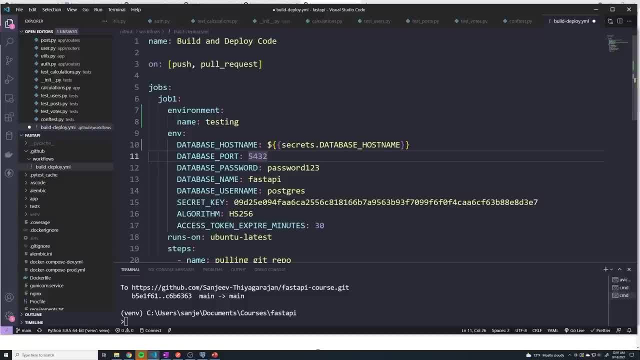 for the repository. I don't actually know who takes precedence. I suspect it's probably the environment, but you should check the documentation to verify. But we don't have any global secrets. I'm going to be using environments for everything, So this keeps things nice and simple, And so now. 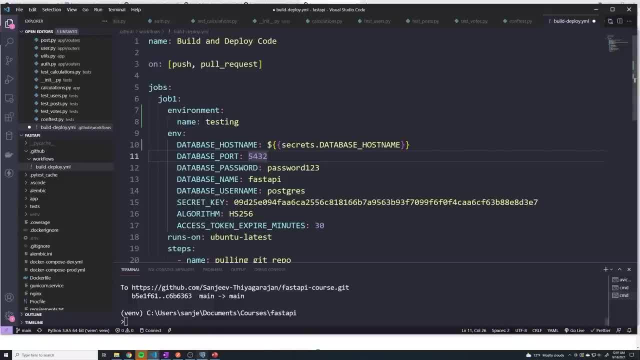 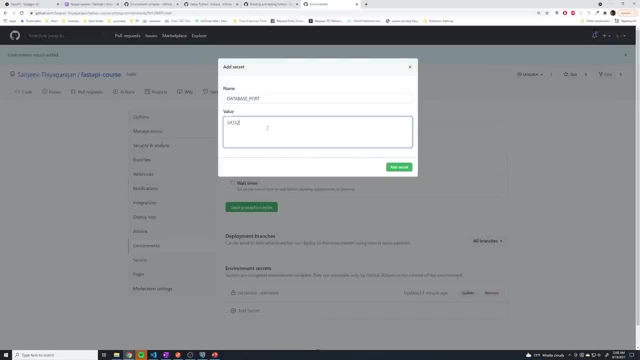 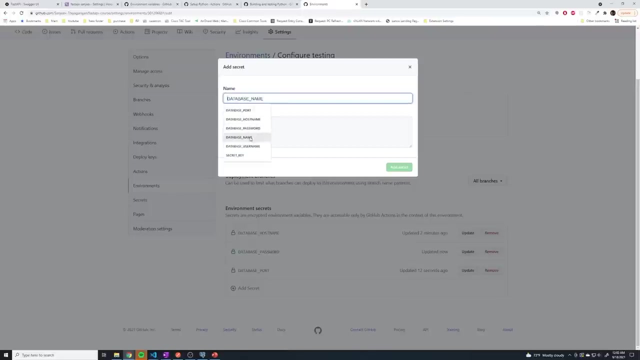 that we've set up this one. let's go ahead and just set up all of these while we have the option, And so we're going to set the port as well. Here we'll set the password And we've got the database name, which we'll just say fast: API. 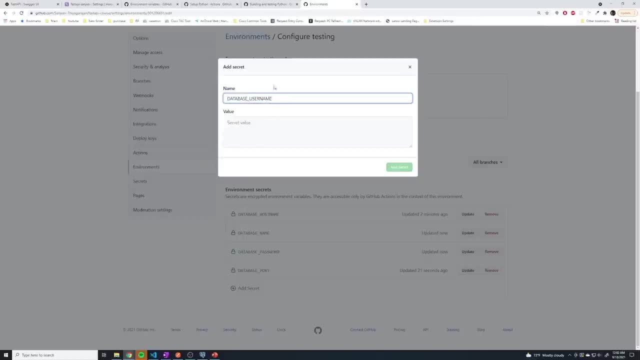 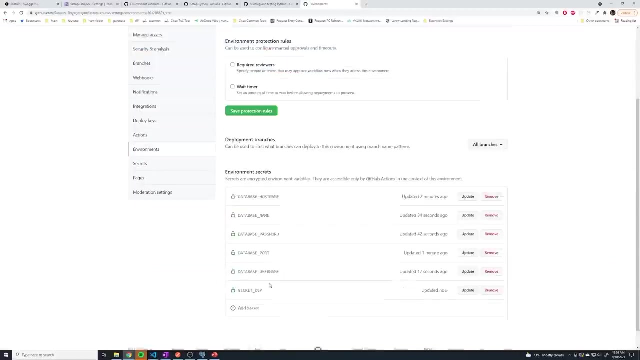 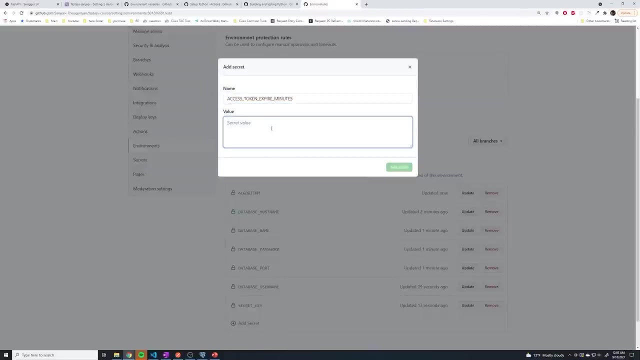 Then the database username and auto filter, because you know, I ran through this all in a quick trial run before I started recording, So it's kind of cached in there And then we're going to go ahead and run the test, All right. and so now that we have all of our environment variables or our environment secrets, 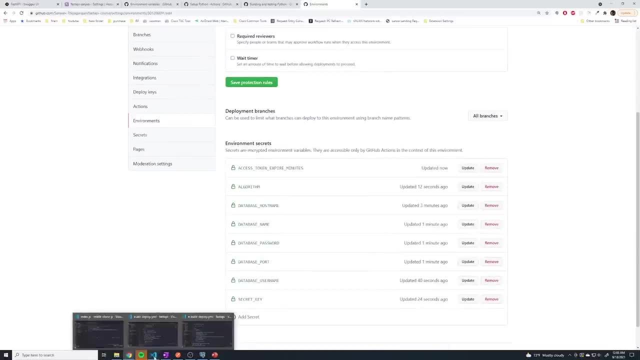 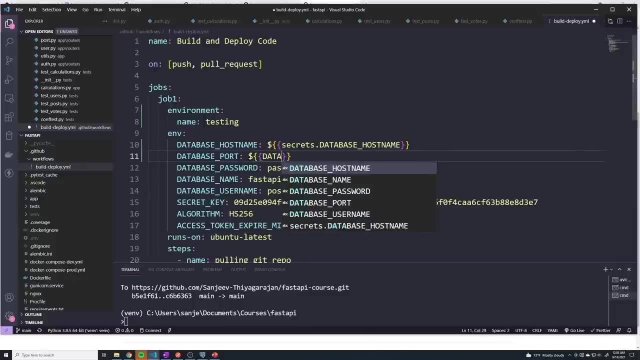 set. we can just change all of these to reference those secrets. we just do the same process And in this case it's just going to be the same exact name as the- the key in this case- And then we're going to go ahead and run the test. 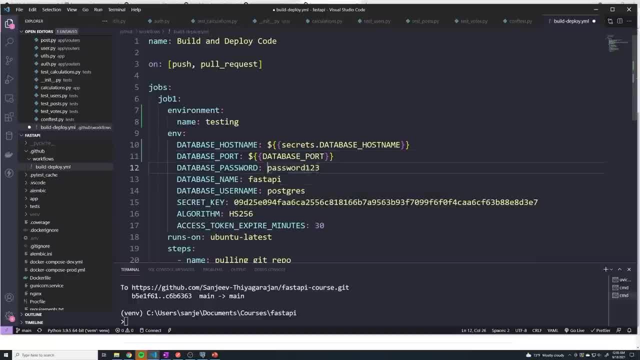 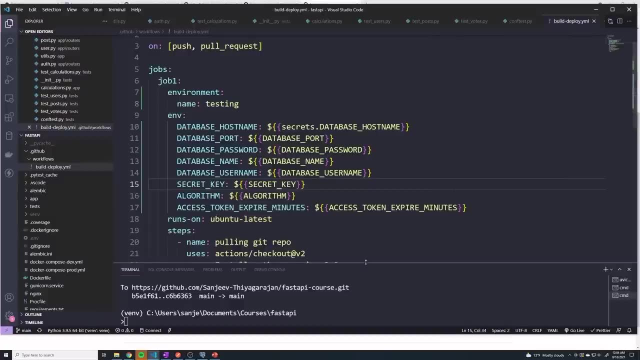 And then we're going to go ahead and run the test, All right, and so now that we got all of these set, let's just save this, and I'm going to check this into git now, just to make sure that you know. everything is kind of working so far. 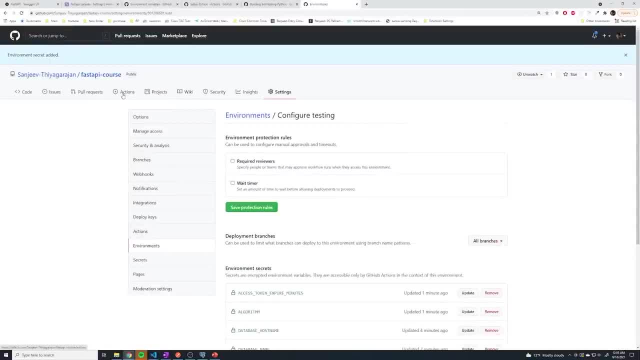 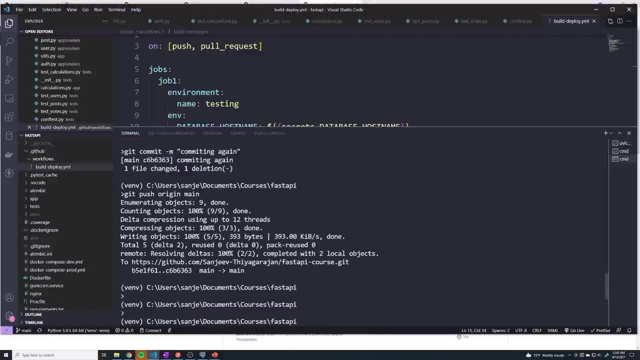 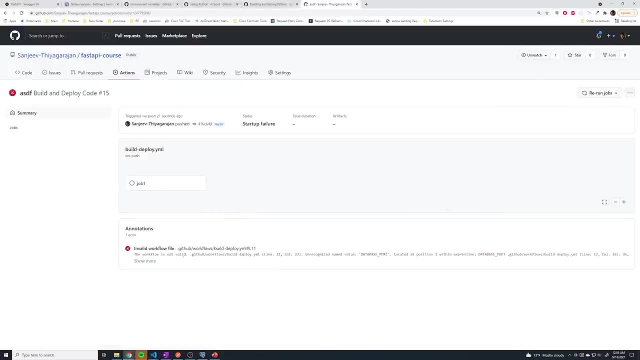 And we'll take a look at the job real quick And hopefully there's no errors or only errors that we expect to see. And what did I call this one? I'll see, I know. Asdf, Asdf, okay, so it looks like it failed already. So we clearly did something wrong. 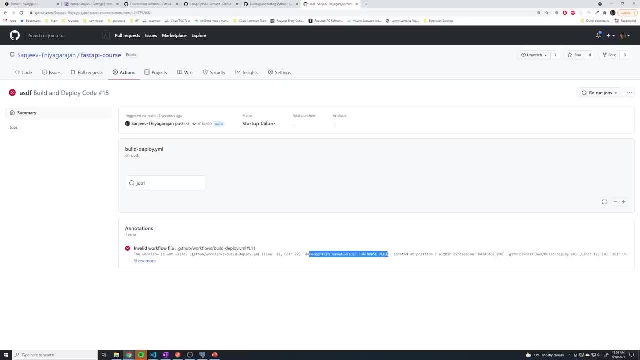 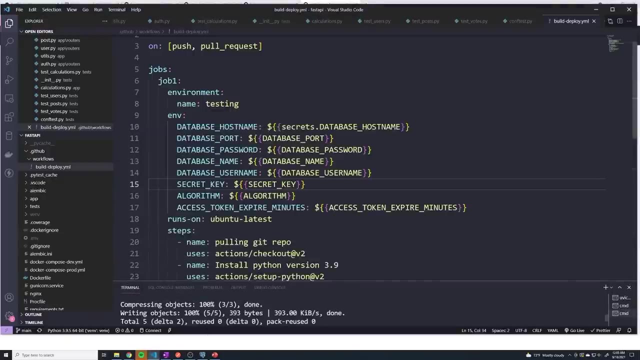 This workflow is not valid. Unrecognized name database underscore port. Well, what happened there? And it even tells me the position. So, if I just like show more database underscore password. so let's see what did we mess up? Yeah, simple mistake. 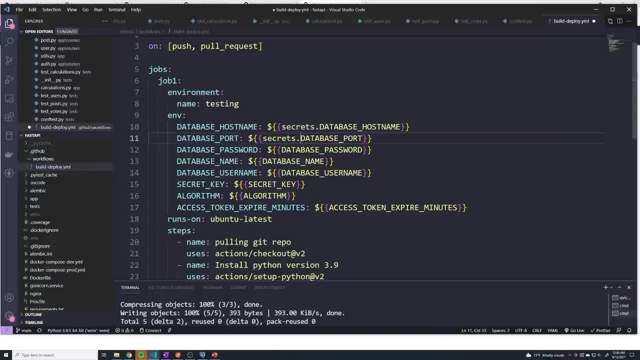 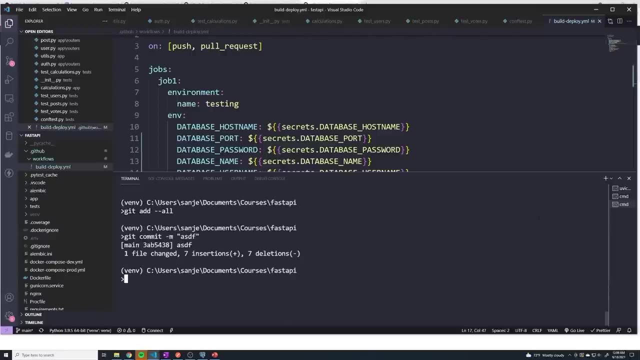 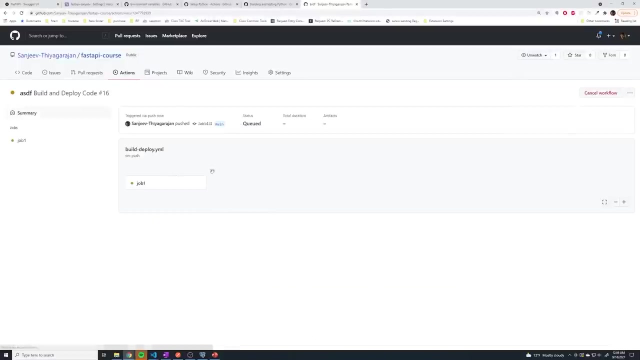 I forgot the secret dot before all of my very variables, So that's why it had no idea what that was. we have to reference secrets to actually get access to them, And now let's try this one more time. Right, this looks. 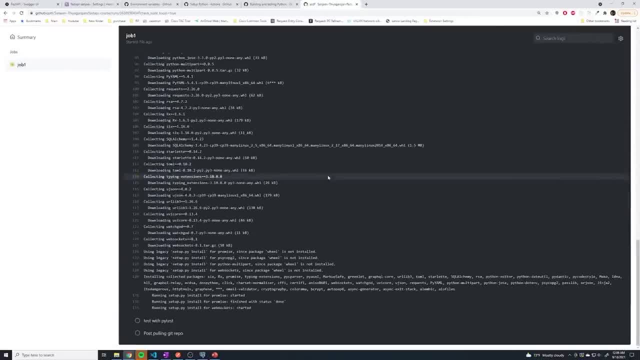 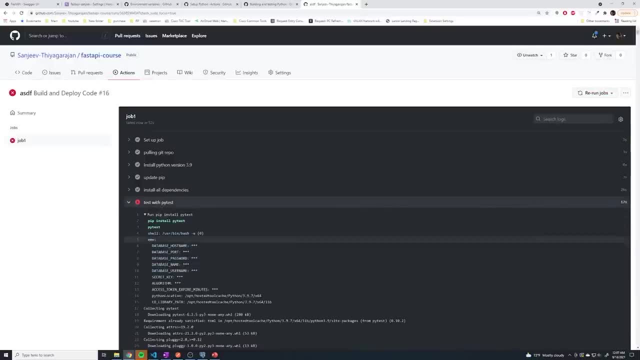 a little better. Alright, and so now if we look at the test with pi test, you can see that the environment variables were passed in, and GitHub will automatically kind of hide what all of the very the secrets are, because once again they're secret, so you shouldn't. 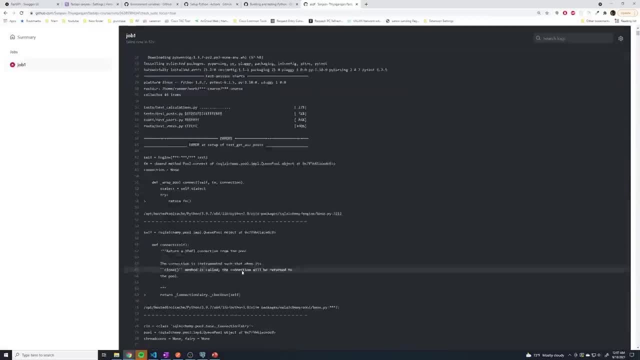 see them, But it does show that we were successfully able to retrieve them. And we got the same error down here. this is just an issue with accessing the database, because there is no database on on localhost. Okay, so now let's try this one more time, All right, so now, if we look at the test with pi test, we can see that the environment variables were passed in and that we're actually able to retrieve them. Okay, so now let's try this one more time. All right, so now we're actually able to retrieve them. All right, so now we're actually able to retrieve. 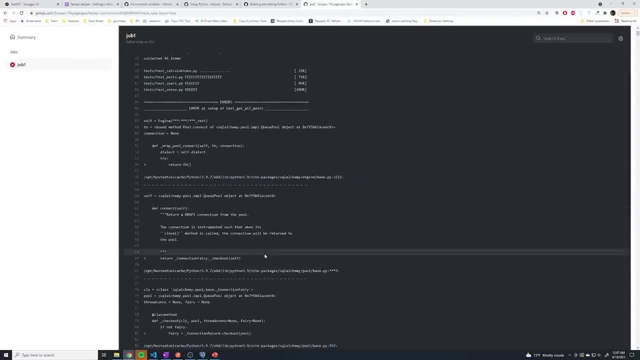 them All right, so now we're actually able to retrieve them. So it's trying to connect to a database that doesn't exist, which is going to create all sorts of issues. So in the next video we'll figure out what we can do to set up a test database on our runner. 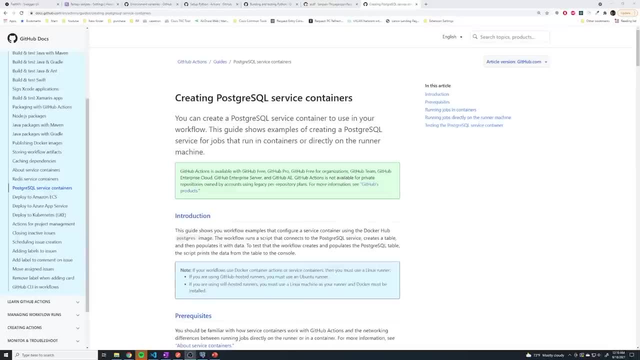 so that we can actually run our tests. So, when it comes to setting up a database on our runner, the easiest way to do that is to create a service container. So what's going to happen is GitHub actions is actually going to allow us to spin up a Docker container. 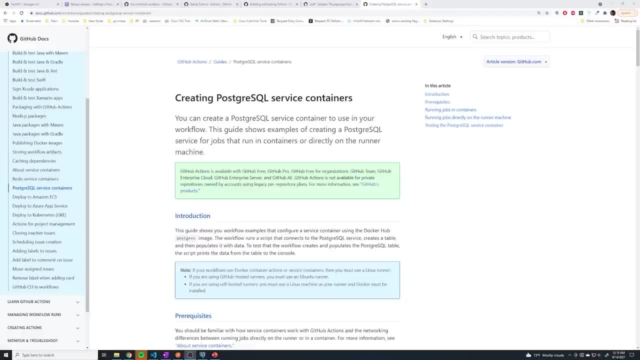 which really is the easiest way to set up Docker on- sorry, to set up Postgres on a remote machine. That way we don't have to worry about any issues with potential installation of a Postgres database, And so I recommend you take a look at this tutorial which kind of walks you. 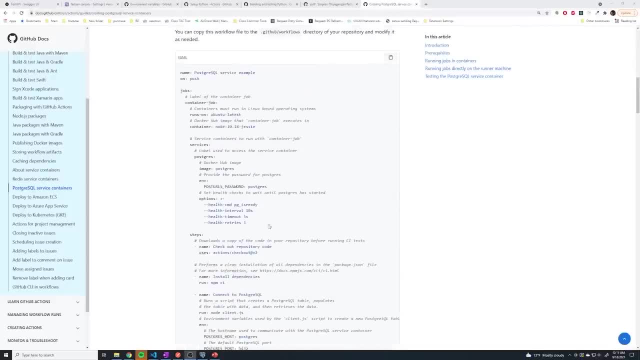 through how to set up a Postgres service container And it just gives you an example, in this case, which we are essentially just going to copy in this case. But here we just under jobs, we specify a service, we give this service a specific name or label, And then we just tell the image. 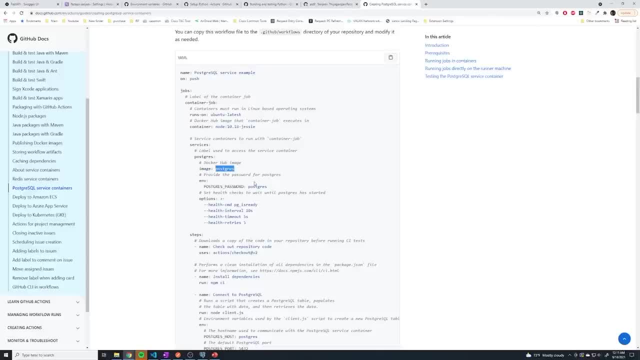 that we want to use, And in this case we're just using the default Postgres image. This is the one that comes from Docker Hub, by the way, But you could technically use any image that you wanted to, but it's Postgres, So we might as well just use the default one, And then we can pass. 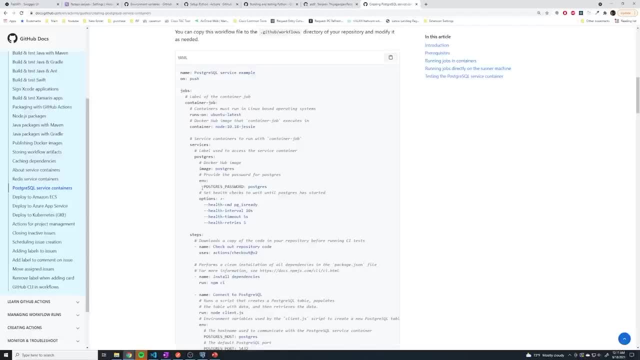 environment variables into the Docker container as well. So one of the things that we want to do is set up the password for Postgres, as well as even, potentially, the database name, And then what we want to do is we want to set up some health checks. to wait until Postgres has. 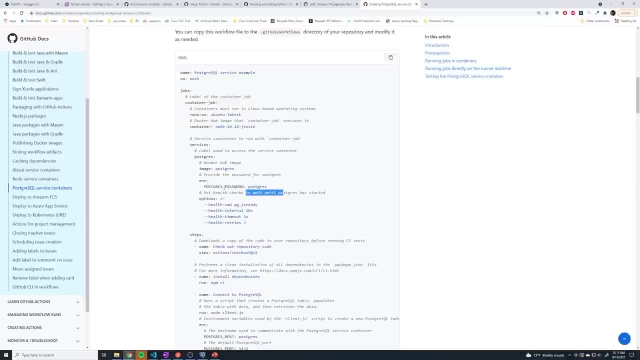 started because until Postgres starts, we should not run any tests, because the tests are going to fail, because the database is going to fail. So we want to set up some health checks to wait until the database is down. So we want to make sure that Postgres is up and ready before we actually 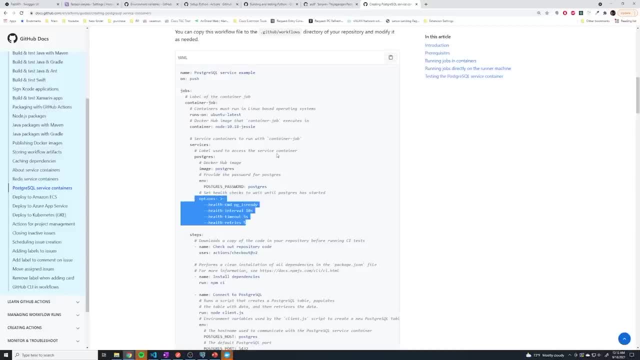 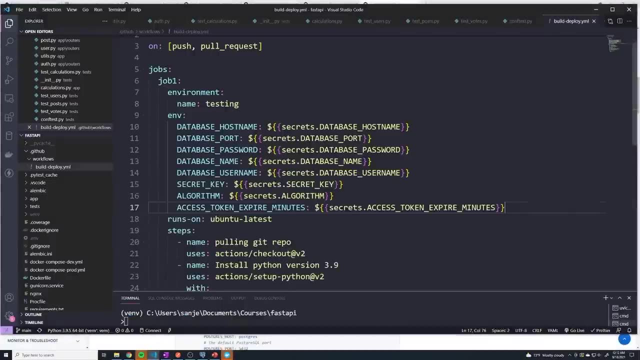 start running our tests. So we're essentially just going to copy this line here. But let's go back to our code And we'll take a look at how to do this step by step. And so I'll just go under the environment variable section here And we'll create a section called services And I'm going to create 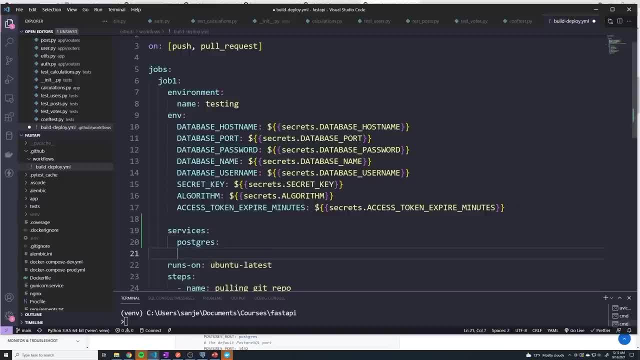 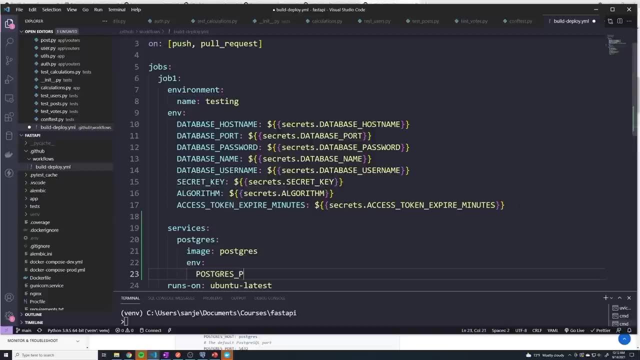 a service called Postgres And we're going to provide the image just like we saw in that example, And that's going to be Postgres And let's pass some environment variables. So the first thing is going to be the Postgres password. So we're going to do Postgres underscore password And here for the password. 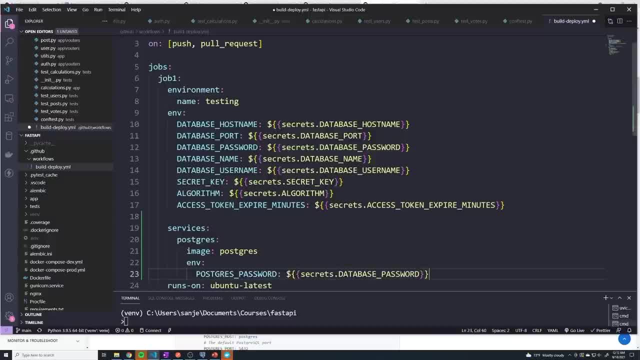 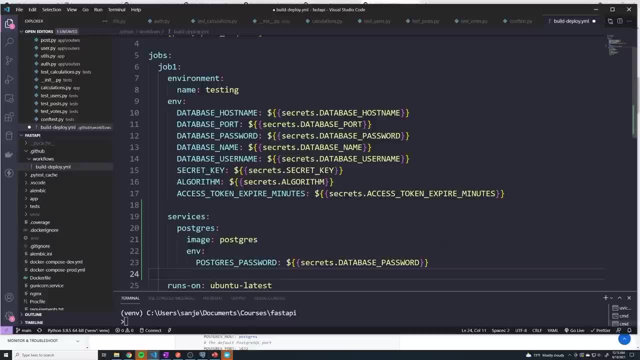 we can literally reference the same exact secret because they're going to be using the same password. And then we also want to give it a custom database name. So we want to automatically create the fast API underscore test database, so that we don't have to do it in code. 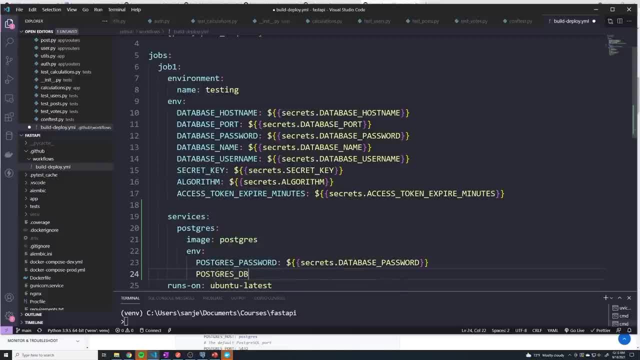 So I'll do Postgres underscore DB And we'll do dollar, dollar, and then here I can pass in where's my database name. So this is just going to be fast API at this point. but we want fast API underscore test Because that's what our code has been set up to run. So we'll do underscore test, right? So? 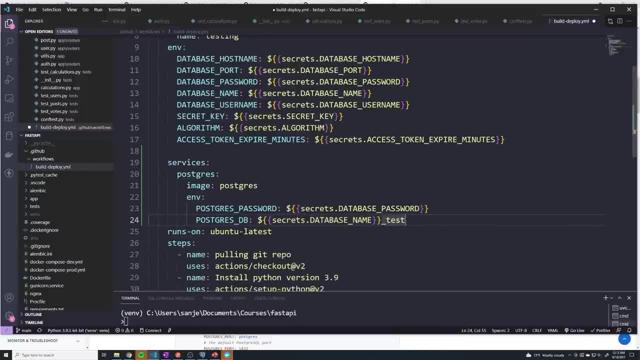 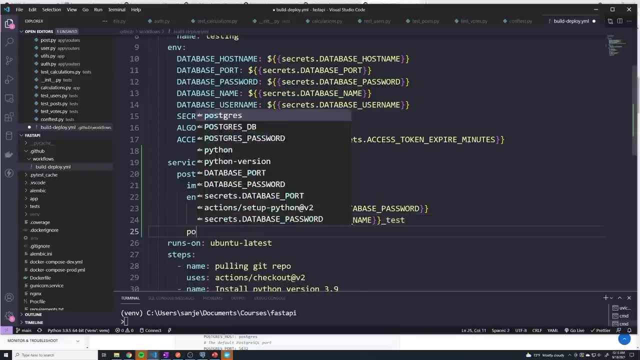 this is kind of like string interpolation, So same thing. And then at that point I think our Docker container is pretty much set up. we do have to specify the ports that we want to open up. So we'll say ports, And you know we want to do. 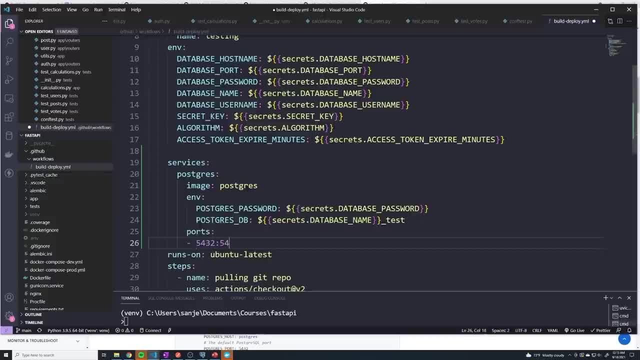 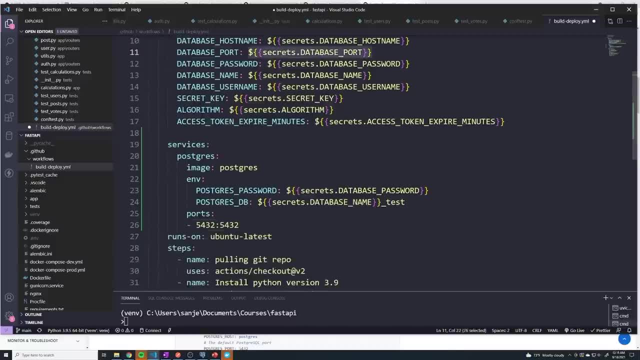 five, four, three, two, and then five, four, three, two. So this is what we want, And you're probably thinking: Well, can we use the, the variables here? and I tried to do this. I tried to paste this here and then paste this here, And I actually got errors. I don't know why it didn't. 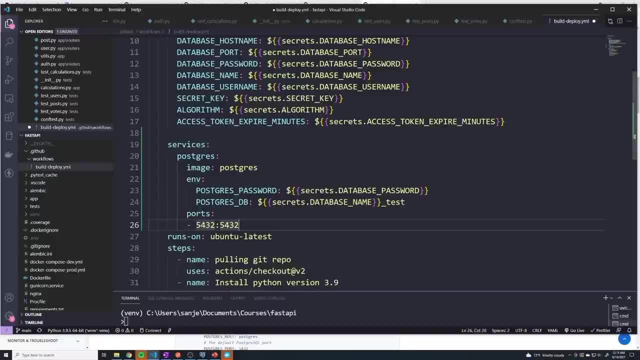 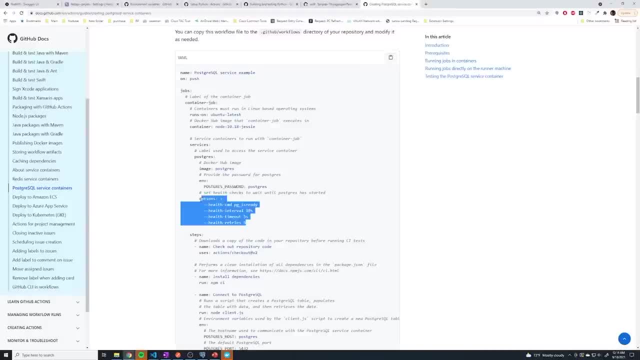 work, But for some reason this wasn't allowed, So you have to hard code these values, unfortunately. And then, lastly, let's set up the options. So I'm going to just copy these options right here, Because we want those health checks for sure. 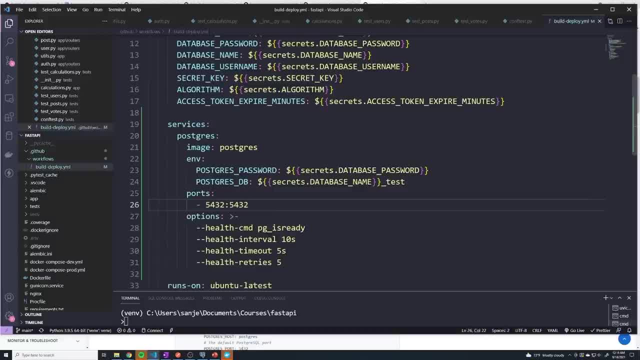 Let's save this and make sure that all the spacing lines up, because a lot of times the spacings can mess up things. I have a auto formatter, So with a for YAML syntax, it'll automatically format it so that all the spacing is set up properly. You want to make sure that you do it manually, or set up or install a. 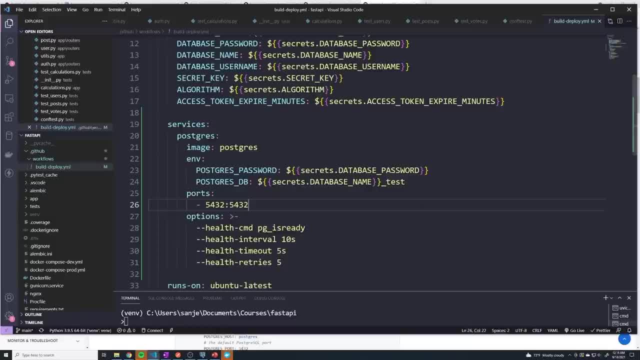 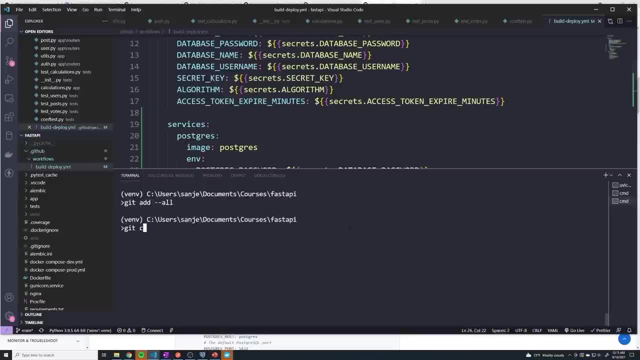 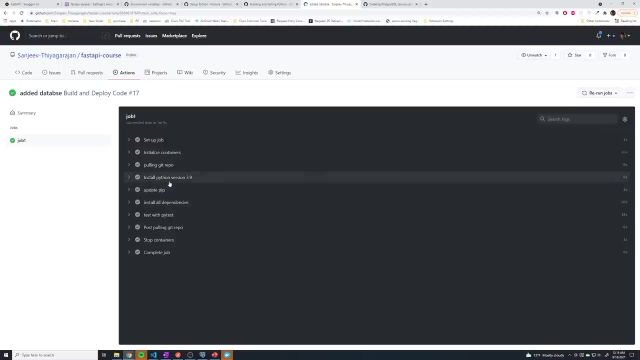 extension in VS code, if that's an option for you. Okay, so we've got our Postgres database And I think we should be good to go, So let's try this: get add all, get commit, All right, And so we can see that our most recent test in this case happened to succeed. And if you 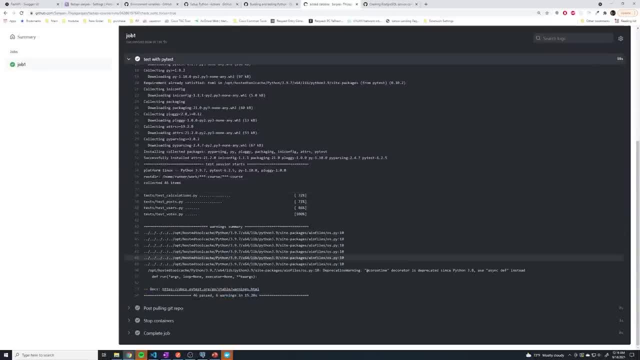 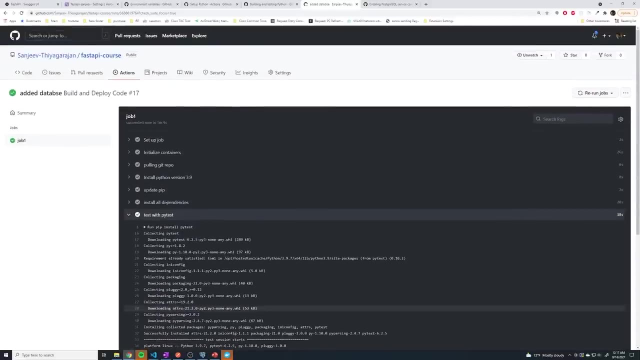 actually go to the test with pi test and just see the results. we could see that 46 tests pass with no issues, And so that means it did successfully connect to our database, And after that it essentially completed the job. So now we've successfully added a database and we've successfully set up our CI pipeline. this is 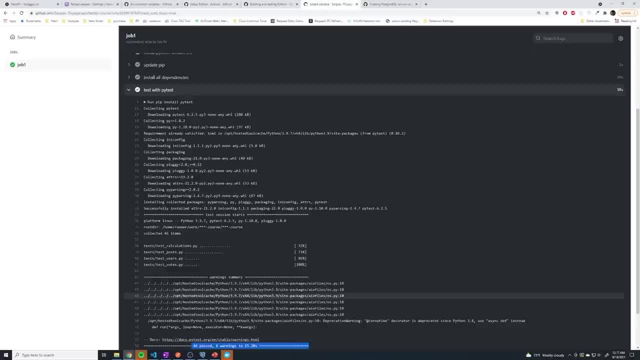 the CI portion of things: to pull our code, install Python, set up, you know, install all the dependencies and to run our tests. So all of this happens in an automated fashion now, just by doing a git push. So you could see how easy it is to get things started. And so, I think, from the CI 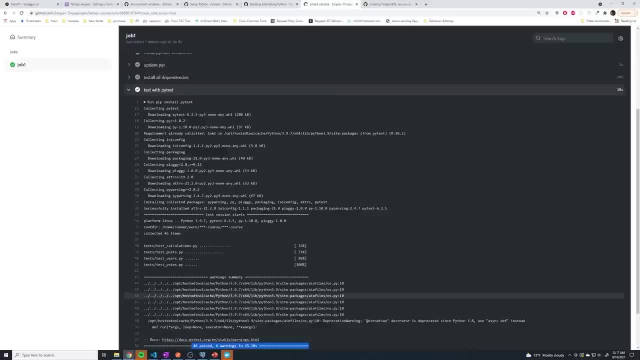 perspective. the last thing I want to show you guys is how to essentially create a Docker image in our runner and push that out to to Docker Hub so that our production network can then pull that brand new image. So there's a couple things that we have to. 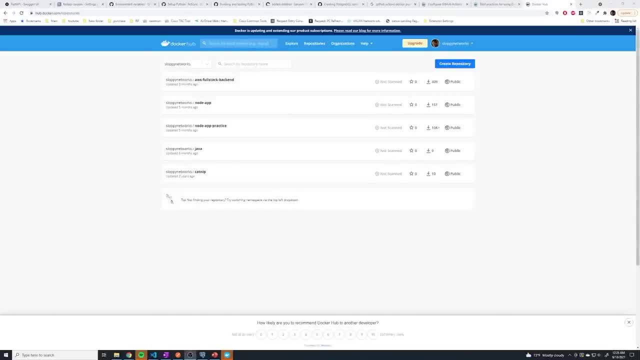 do to get Docker working in our GitHub workflow. The first thing is we need to have a repository setup on Docker Hub to store our images, And if you did not create one during the Docker section, go ahead and create a new one. So log into Docker Hub, select, create repository and just give this. 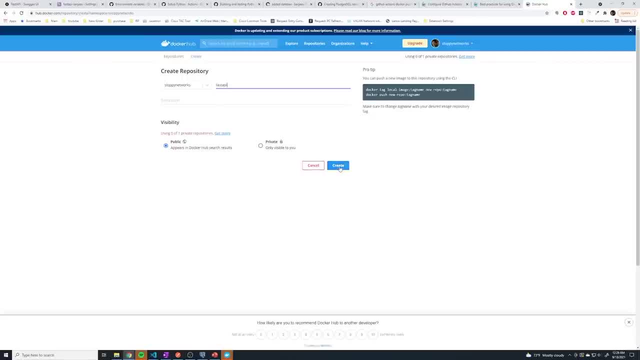 a name that you can remember. In this case is going to be fast API. I'm going to call it that and then make it public, just to keep it simple. And so this is our repo, And then it's going to tell us how to actually push an image to. 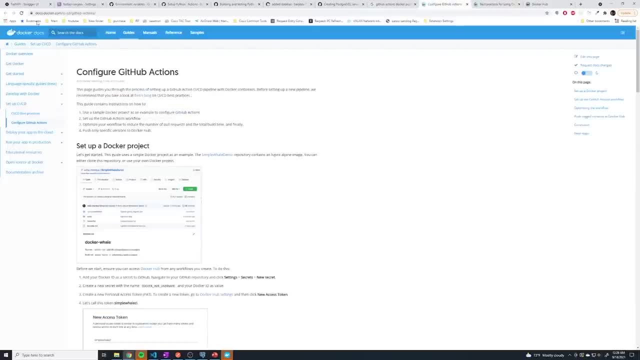 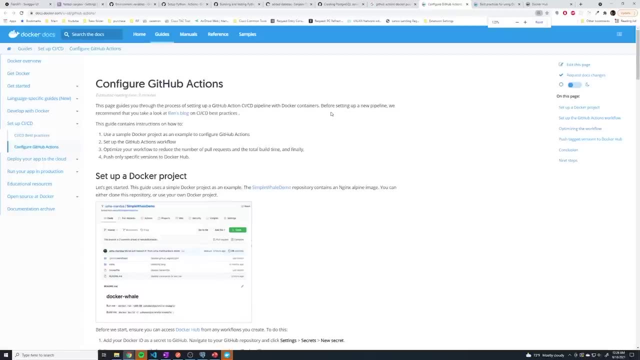 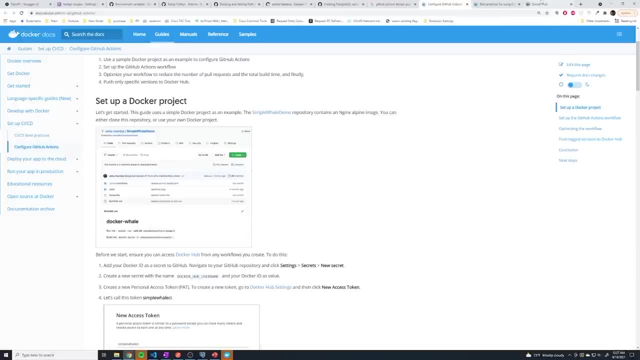 it. And then if you go to this page right here- so docsdockercom, slash, CI, CD, slash, GitHub actions- it's got an excellent tutorial that we can follow for setting up Docker with our GitHub actions. And so if we go back to our Docker Hub, the first thing that we want to do is we want to: 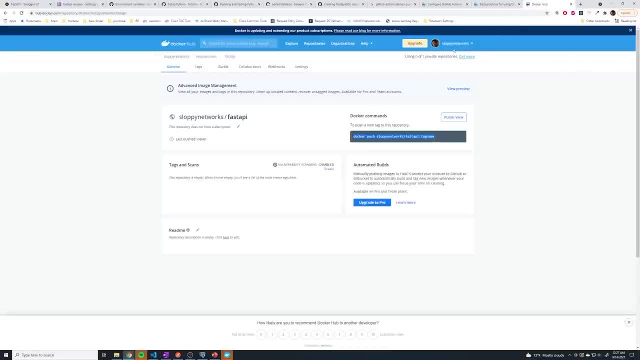 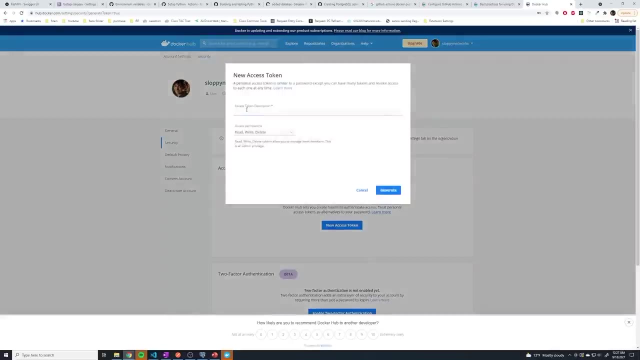 get an access token. So let's go here And I think we go under settings- or well, it doesn't look like it's here, Maybe account settings, Yep, and then security, and then we can select new access token And I'll- maybe we can call this GitHub actions And we're going to give it, you know. 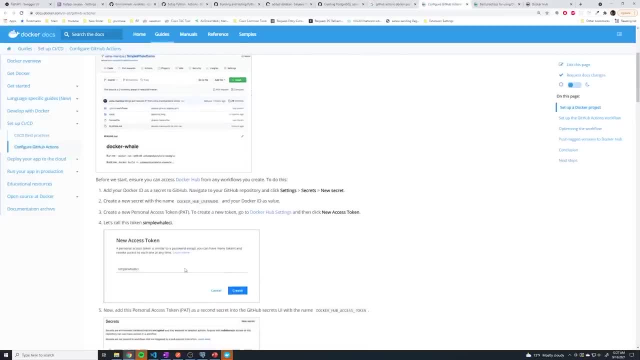 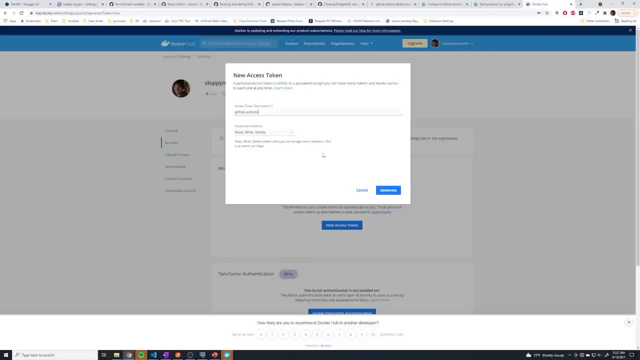 whatever permissions that you want. Does the Docker give us information on what permissions? It doesn't look like it In this case, so just go ahead and select all of them for now. All right, and so it's going to give you your access token. make sure that you don't share this with anyone. 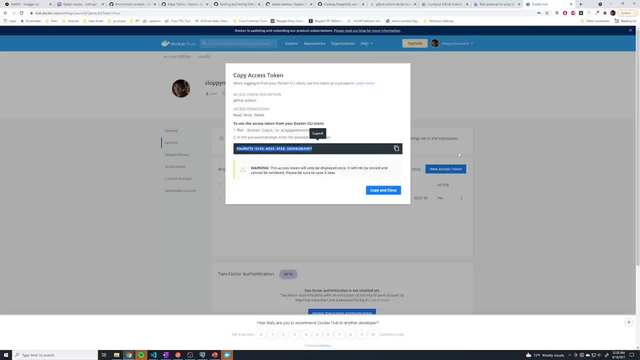 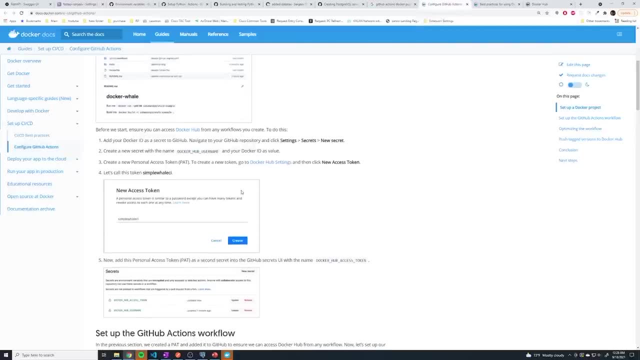 else, And it's only going to be displayed once, So go ahead and copy it and make sure that you have this. Then what it's telling us to do is: we want to create a, a secret for both our users and our users. So we want to create a secret for both our users and our users. So we want to. 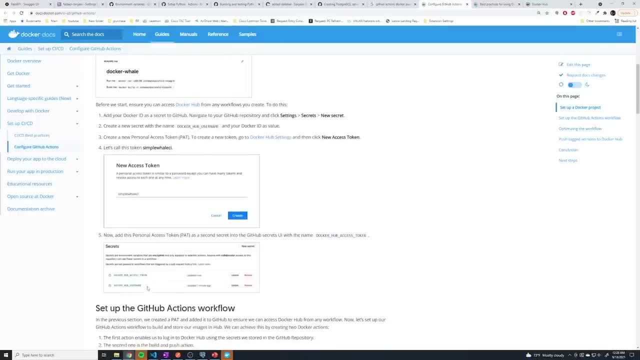 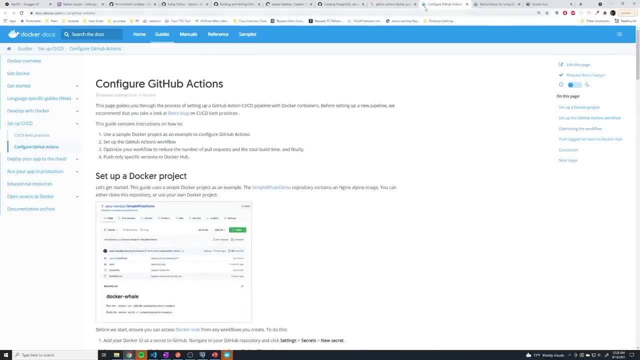 create a secret for both our users and our users. So we want to create a secret for both our users username as well as the Docker hub access token. So let's create these two secrets in GitHub for Docker hub access token and Docker hub username- And I actually forgot what my username was. Okay. 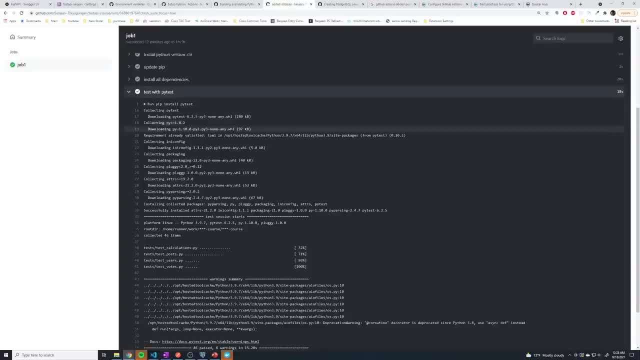 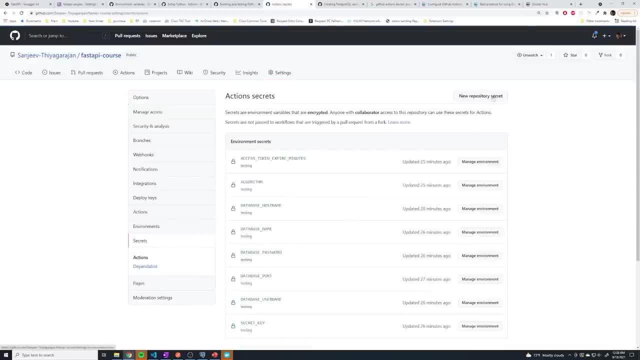 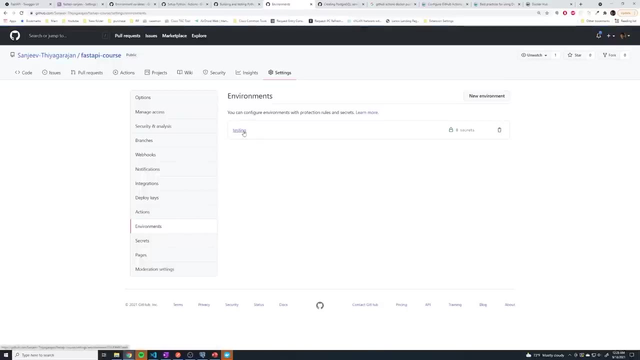 so it's sloppy networks, And so here we'll go into settings And feel free to use either the global repository secrets or environment secrets. I'm going to just put this in the testing environment for now, But you can use either one in this case. 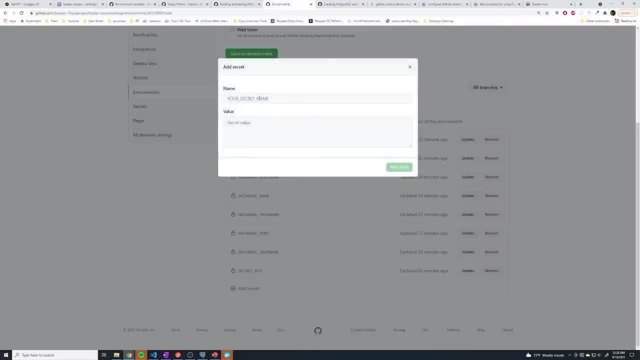 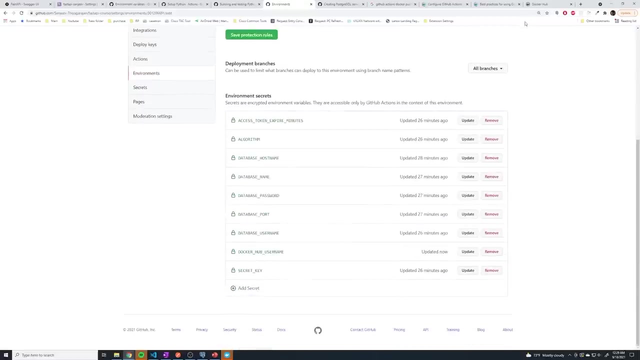 And so we got Docker underscore hub underscore username. So this is going to be sloppy networks for me, but it's gonna be something else for you guys. And the last one is going to be Docker hub. What is it? Docker hub access token. 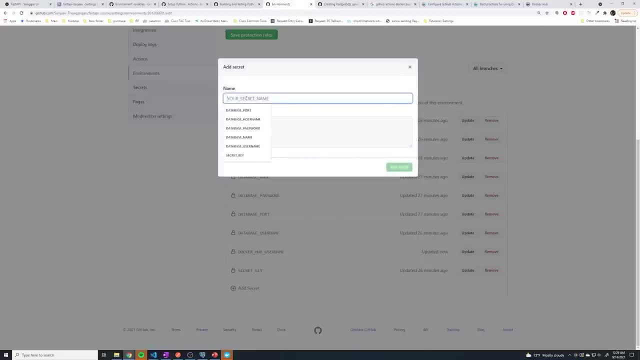 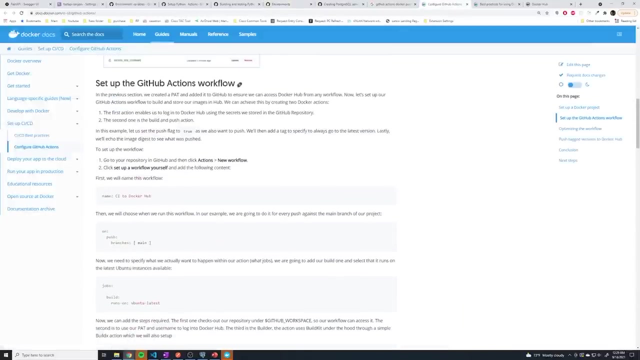 And so we're going to go into settings. And so we're going to go into settings. And so we got Docker hub access token. And so we're going to go into settings. And so we got Docker hub access token. And so once we get that setup, you'll see that they're going to give us the steps on how to actually set. 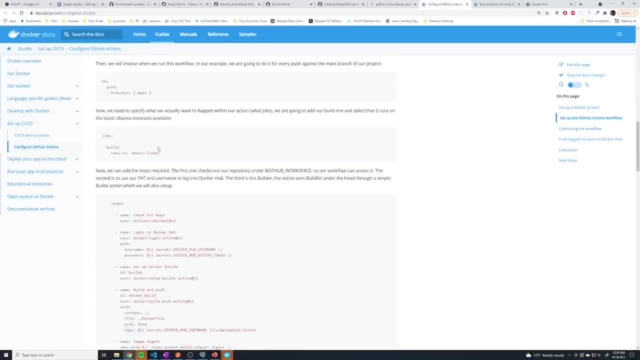 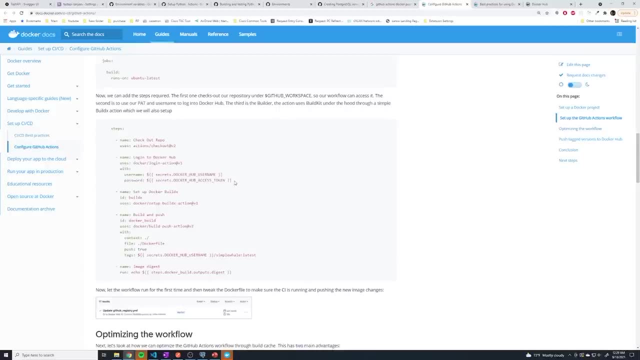 this up in our YAML file. you can ignore the original the the setup process, And what we want to do is we want to go down to the this section right here which shows us how to log into Docker hub. So we can literally just copy this straight up And just paste it in here, So we can just say: 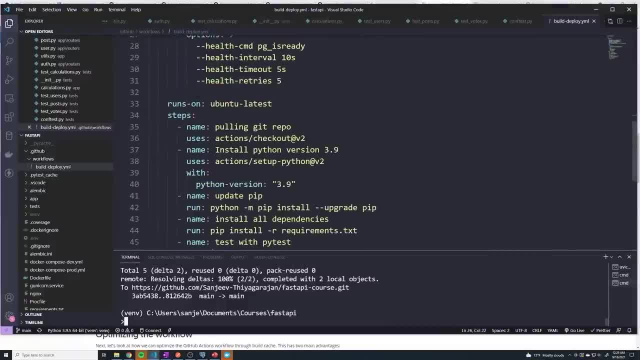 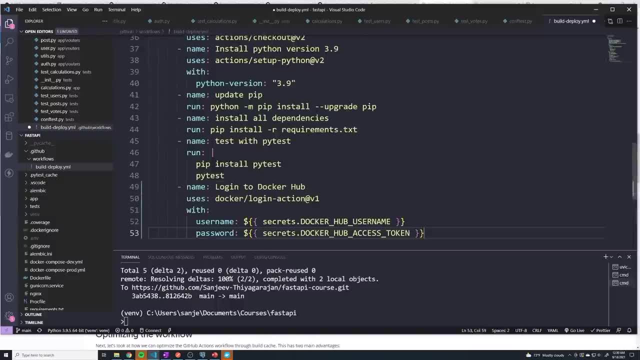 we'll do it at the. what step should we do this at? We'll do it at the end just because- why not? Because some of you guys might not be interested in setting up Docker, So it's going to be an optional step at the end. 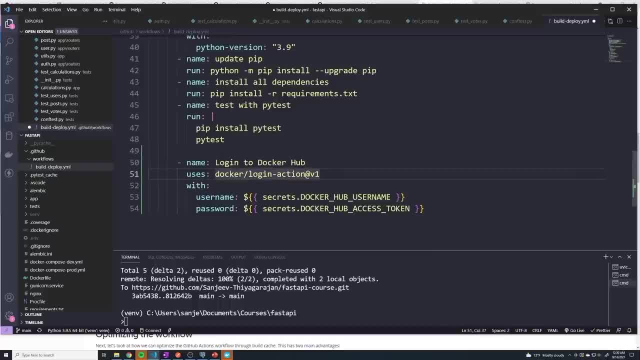 So we'll log into Docker hub using this built in action from the marketplace, And then here it's just going to provide two properties: username and password, which is going to reference the two secrets that we created. All right, and then we want to set up Docker build x. 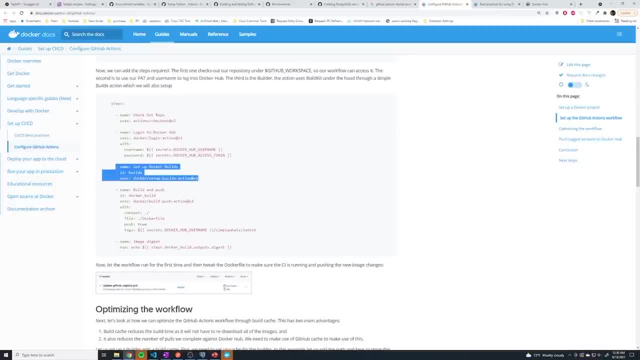 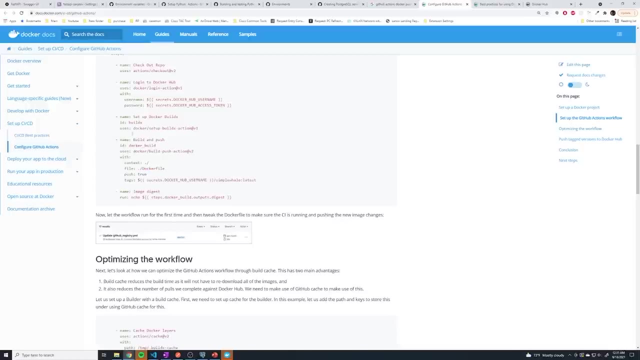 so we'll copy this one as well. All right, and then we have the build and push step right here, which, in this case, it's a, once again, a built in action, And all it's going to do is we're going to provide a path to the context. 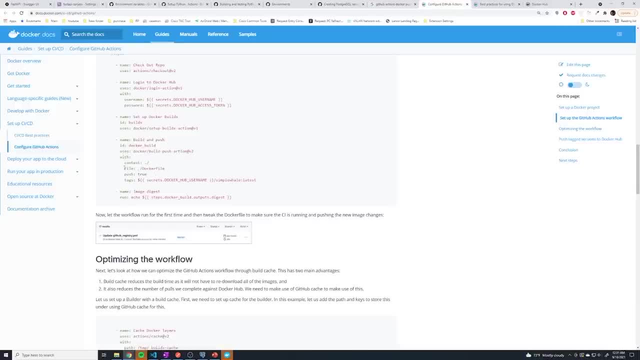 So this is essentially where is the Docker file located, And we I this is technically optional, but if you want to, you can hard code the specific Docker file. I think it should default to this one, because that's the default Docker file, but we'll just put it in, just in case. And then the 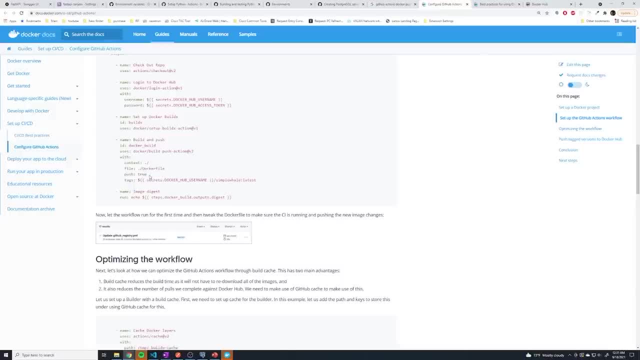 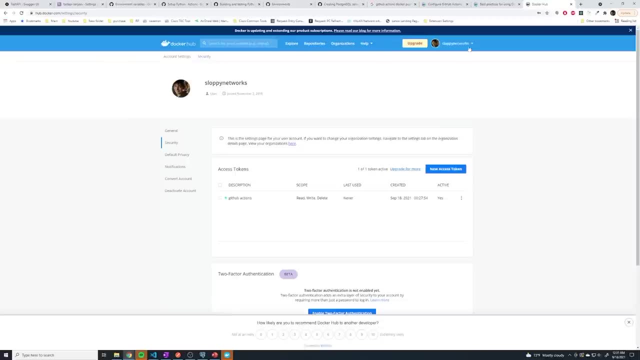 push is means not only are we going to build the Docker image, we're also going to push it up to Docker hub And then we have to give it a specific tag. And if we go back to Docker hub and I go to my repositories and I go to my fast API, it's going to show me the format of the tag that I 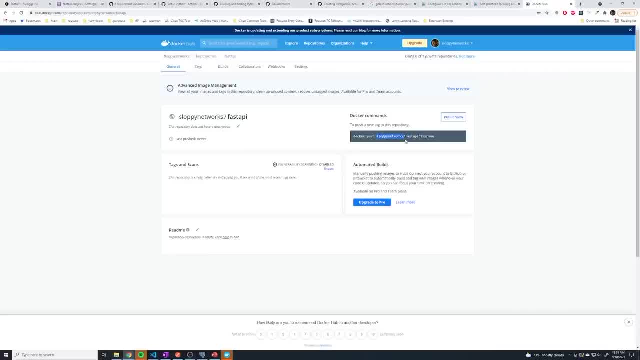 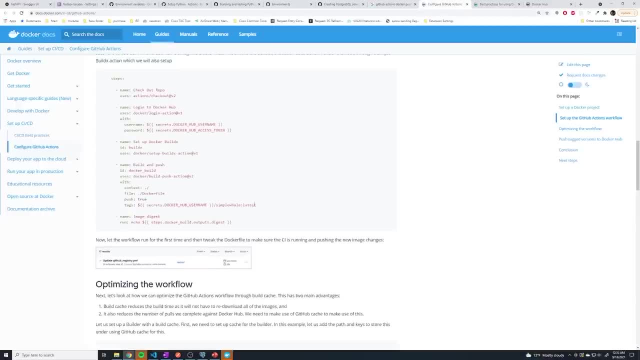 need so that I can actually push it up properly. So it's going to be the username slash, and then the name of the repository, which is fast API, And then we can also give it an optional tag name as well. So once again, we're going to copy this and just update a few fields. 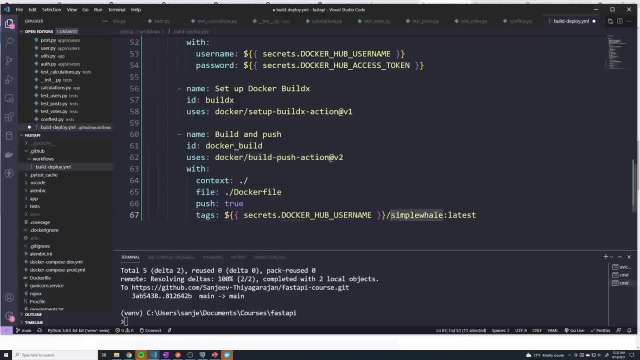 Everything else should be just fine. The only thing that we have to change is this is going to be fast API and it's going to reference the username, So it's going to be in the exact format, And if you want to give it a very specific tag, you can give that as well, but I'm going to just 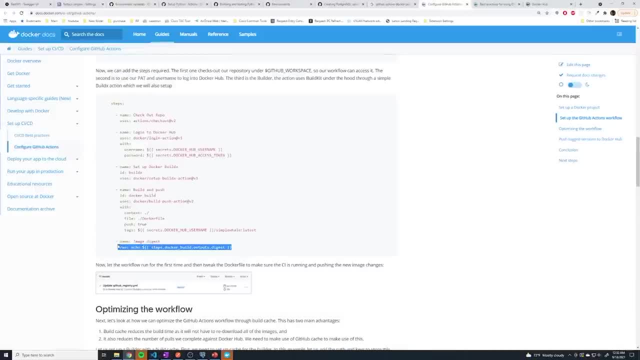 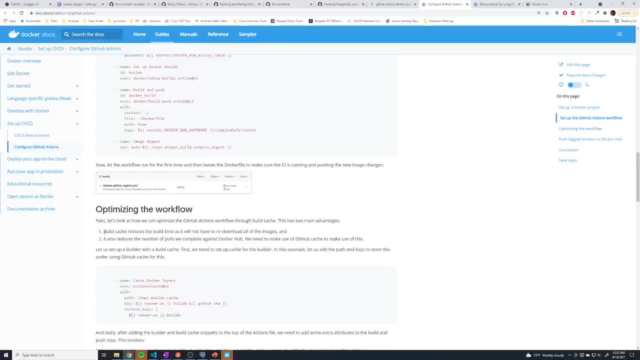 give it the default latest And then here it's just printing out The image digest, which is, for us, is optional. You'll see that it does provide us some optional things that we can do for optimization. So we can use the build cache so that we don't have to redownload all of our images every time we run. 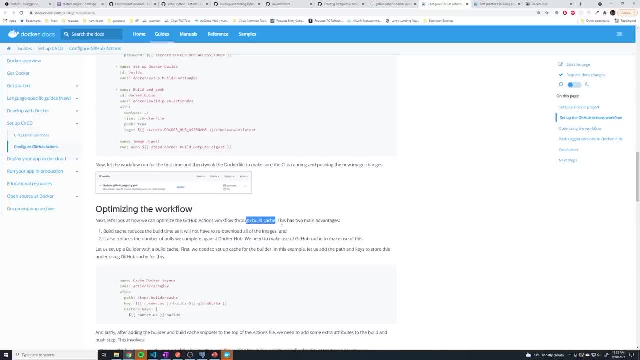 because that's going to extend the build time and the runtime for our runner, which is eventually going to cause us a certain amount of money. So this is the code that you can use And if you look at the bottom right here, this is going to show us all of the 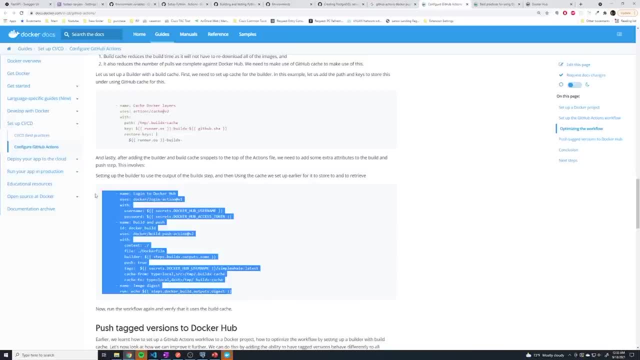 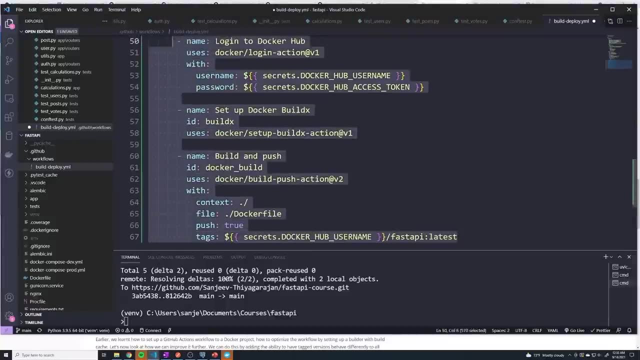 code at the very end. So we can literally just copy all of this if we wanted to and just use that instead of what we put. So that's what we will do. So let me just delete all of this And then paste it in. 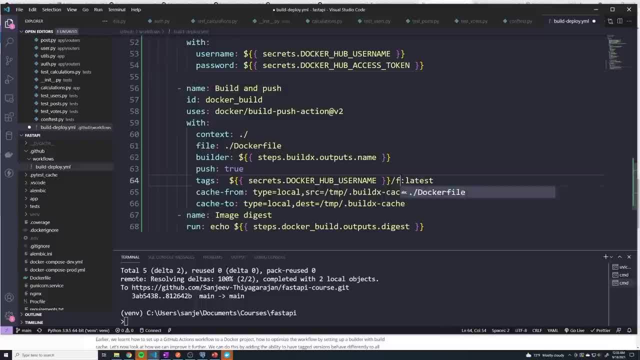 And we have everything. And once again, we just want to change the name to be the repository name, which is right here. we can also use a secret for that, But don't worry too much about that. And that should be all that we have to do for the Docker integration. If you don't have a Docker, 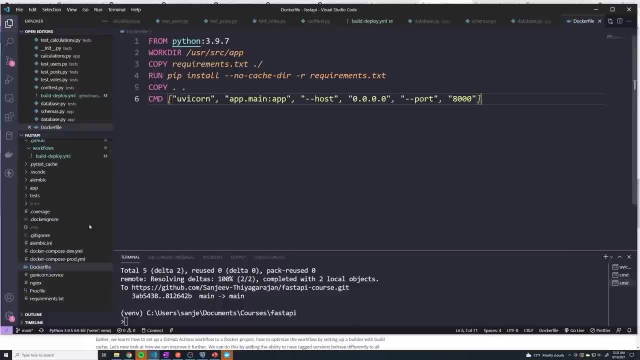 file, then I'd recommend you- Well, I'll just pause this video- create a file in your root and the root of your project directory called Docker file, with a capital D, And just copy all of this, or you can follow what I go through in the Docker section if you guys skip that. 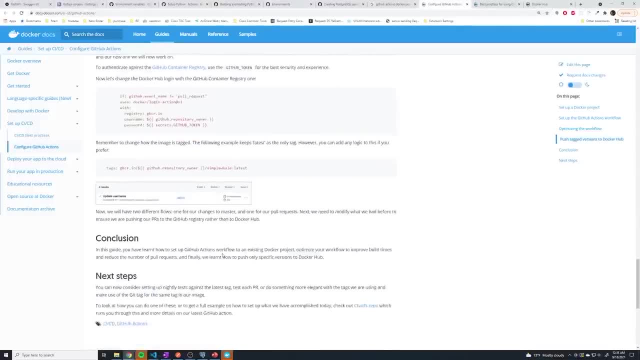 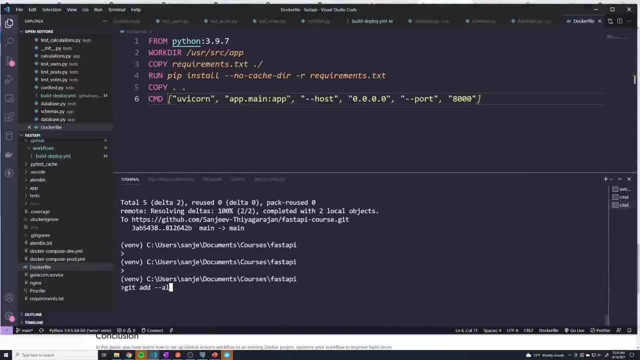 And I think that should be everything that we need. So let's go ahead and push this And pray that it does not break anything And it works just the way we expect it to. So we'll do get add dash, dash, all get commit, added Docker, And then we'll do a get push origin. 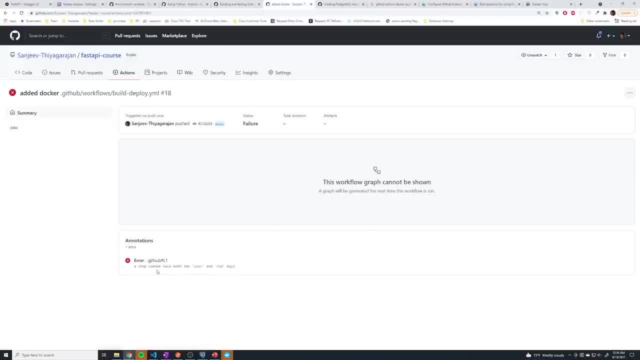 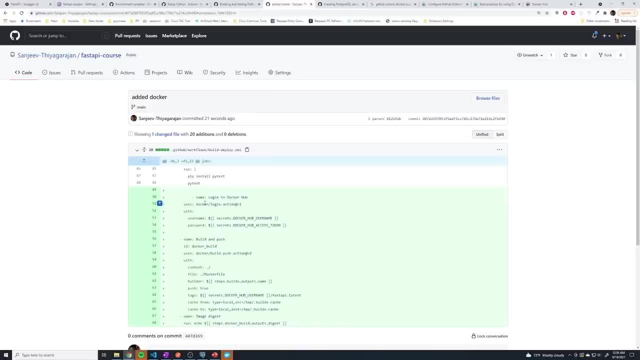 Yep, and it failed, So fully expected this. A step cannot have both uses and run key, So what did we break here? Actually it should. Where is it telling us this? Yeah, this spacing got messed up, So that was a. 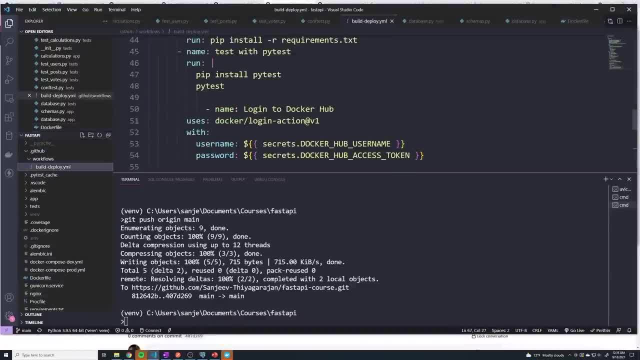 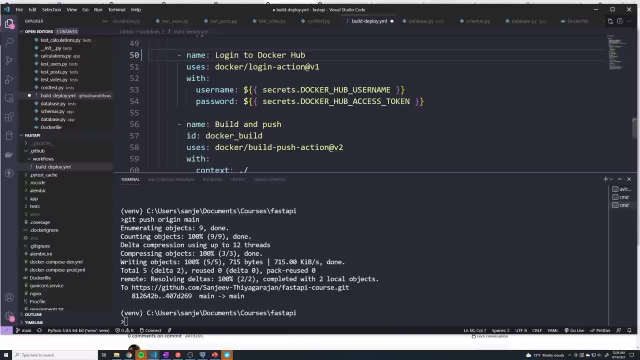 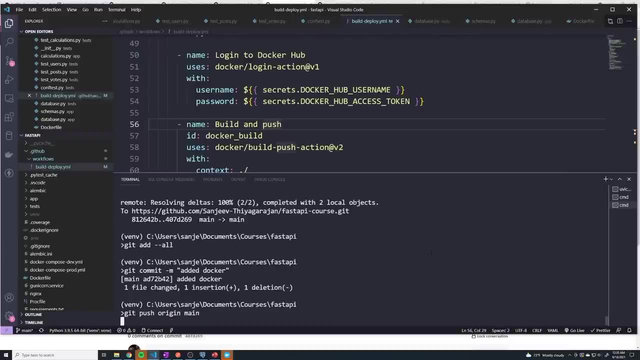 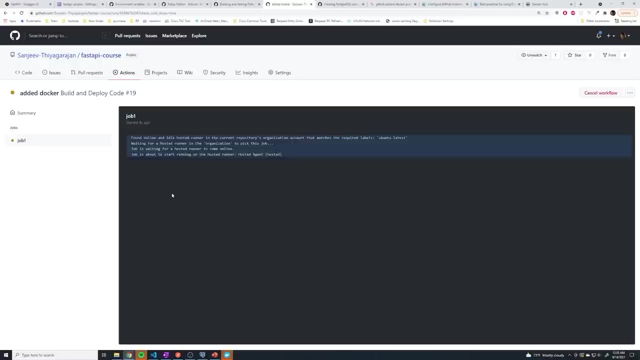 very obvious mistake that I should have caught. I just have to move this back right there And that should fix everything. So let's do this again. All right, so so far it's not erred out. So it looks like things look okay. 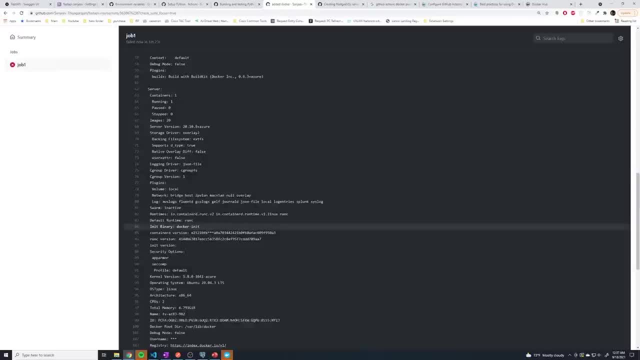 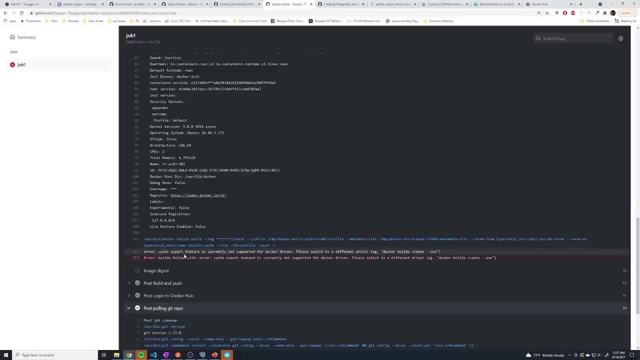 And we can see the build and push section failed. So let's see if there's an error. And it looks like the there's some issue with the driver. Please switch to a different driver. Docker, build x, create, dash, dash, use. So let's see what the error is. 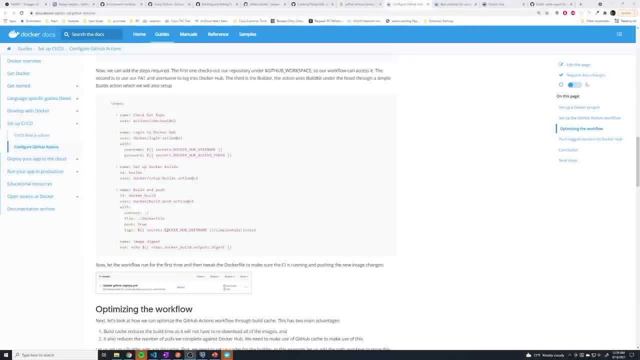 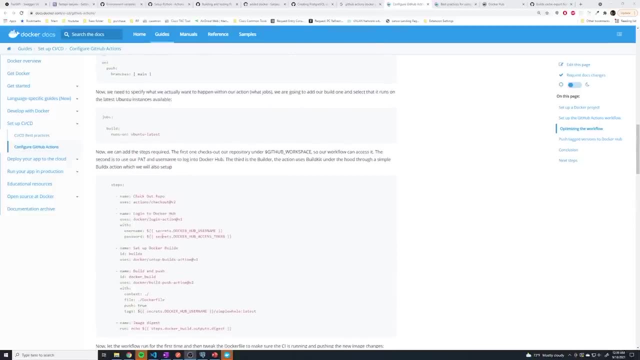 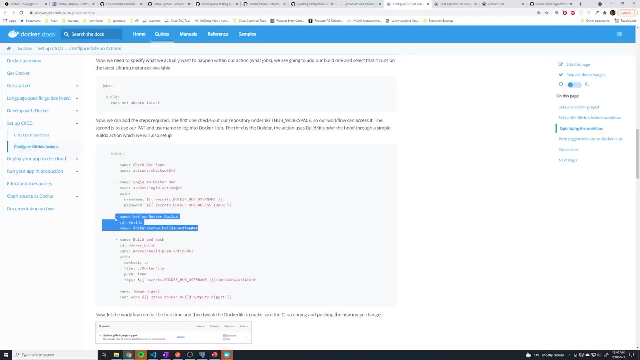 All right, so let's see what that is in this case- And I realized the documentation was a little confusing- this section that we copied at the end, It didn't include one of these steps, which is the build x step. So before we are actually, after we log in, we want to set up a build x, which is the mistake that we ran. 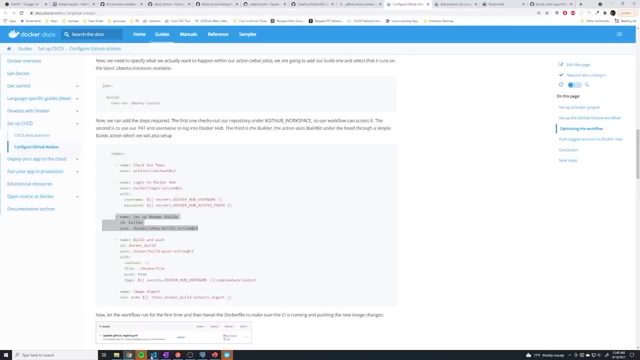 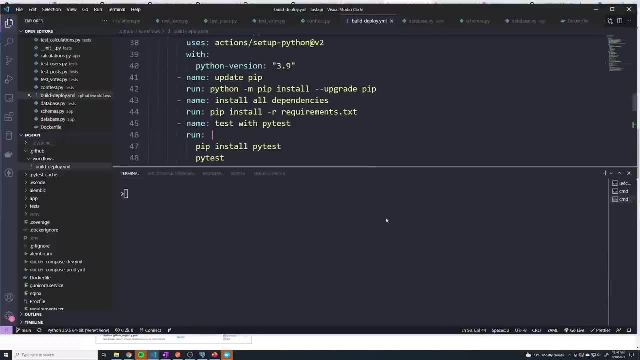 into. So we want to copy this page right here, this section, and then we'll run that right after the login. And so now if we do a git, add all Git, commit, dash, m And then a git push origin main. 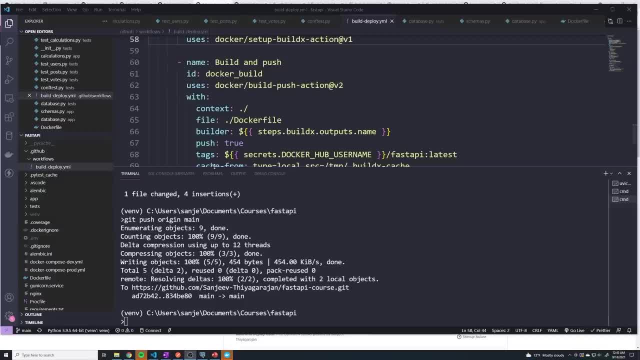 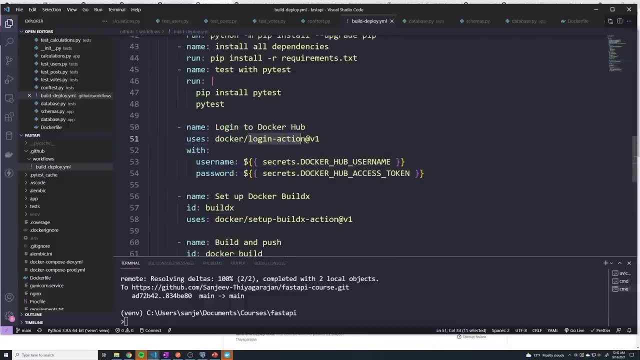 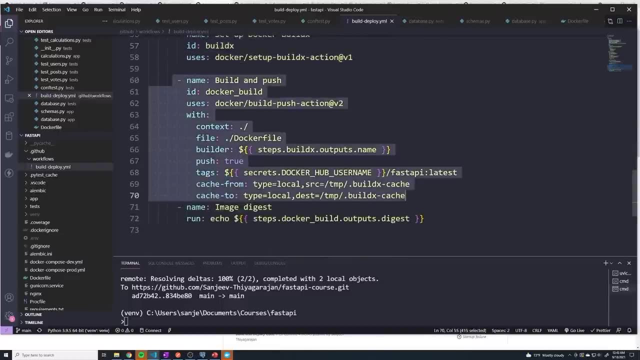 Okay, so I think this time everything should work. But just to reiterate, because I think I went a little bit quickly, the steps are: we first log into Docker using the login action right here. Then the next thing is: we, we used, we set up build x, And then we call the build and push action in this case, And 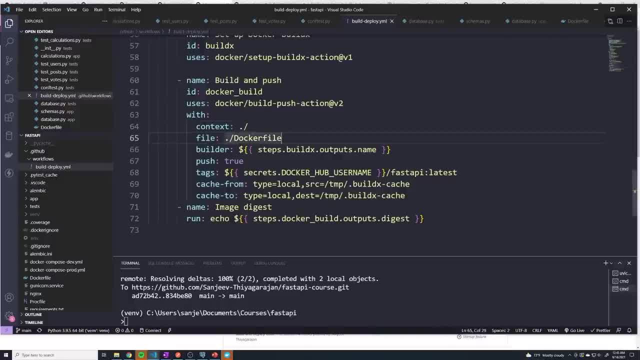 here we specify the context, which is saying just this current directory, and then the location of our Docker file, And then we're going to use build x for the builder And we set push to be true because we want to actually push it to the, to the GitHub repo. 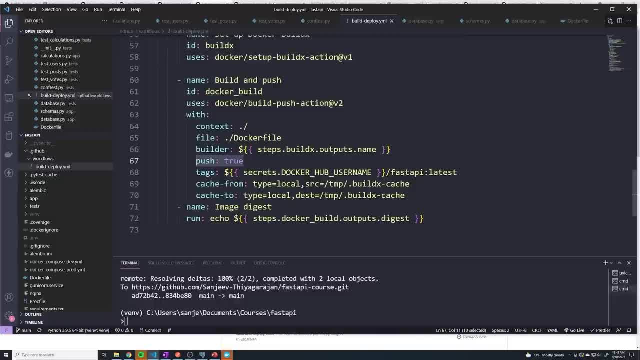 And then here the repo is going to be our username slash, then the repository name, which is happens to be fast API. we could store this in a secret, but I decided not to. And then these are just copied from the documentation so that we can cache all of. 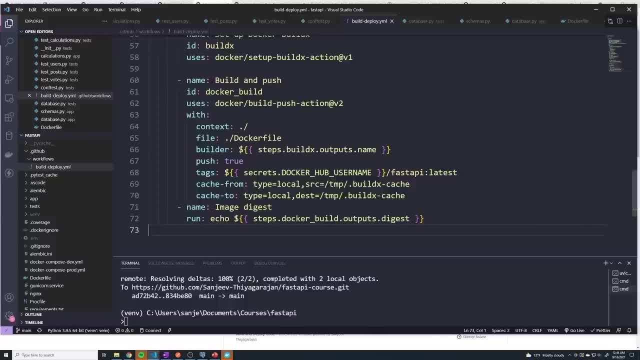 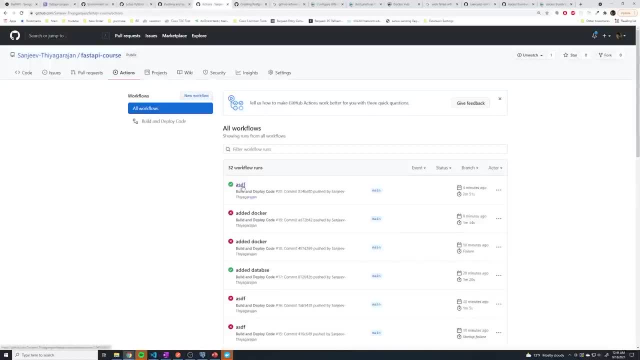 the images so that we don't have to keep running all of this from scratch, which is a fairly long process. And then here we're just spitting out the image, digest, And if we take a look at our workflows and we can see that the last one, which is called ASDF, 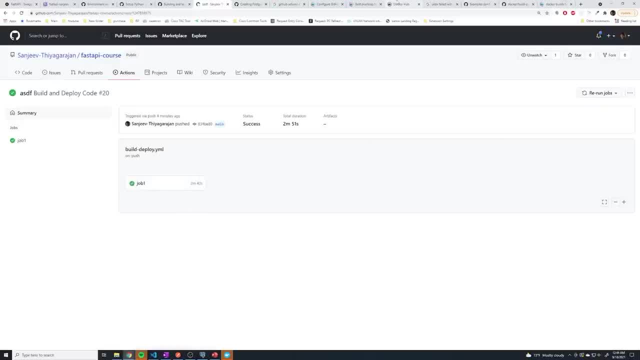 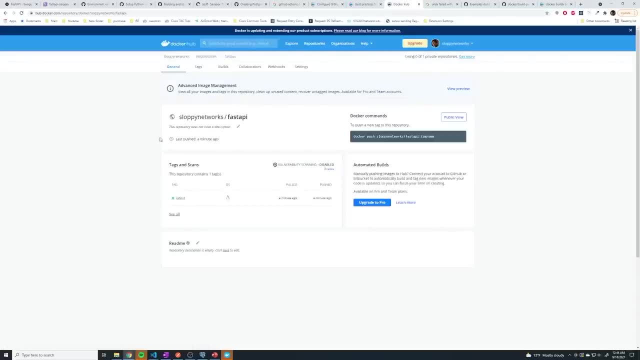 successfully ran. And if I actually go back to my Docker hub in this case and just hit refresh right, we can see that we did successfully run our Docker, successfully push an image a minute ago, So that means we have now successfully completed. 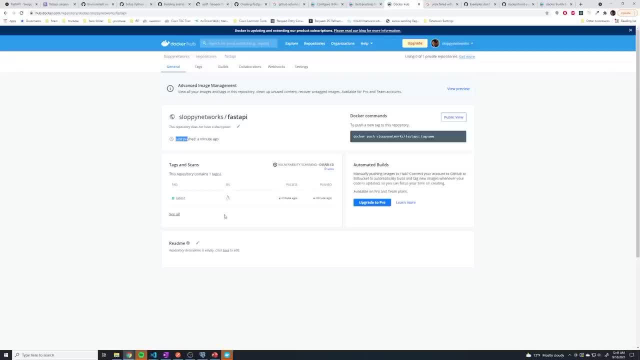 our entire CI portion of our CI, CI, CD pipeline. The next step is to set up the continuous delivery, which is a matter of just providing a whole bunch of commands needed to actually push out our new code to our production network. And you know, moving forward just to kind. 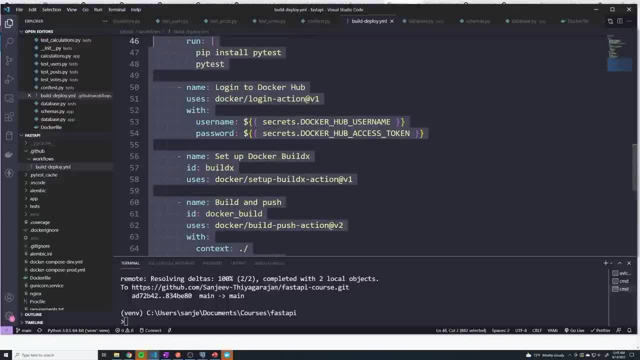 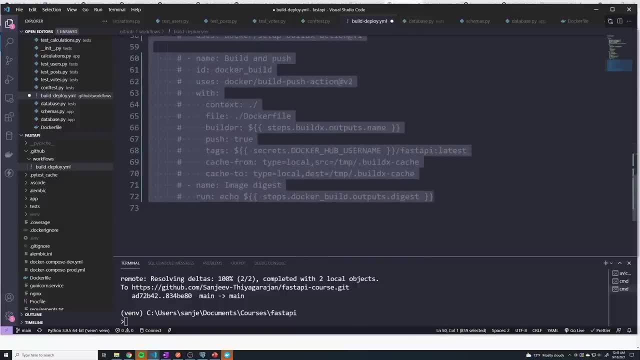 of keep things simple and as quick as possible. I'm actually going to copy out all of the Docker steps, Because we're not even using Docker in production, So we don't actually need this. So we'll just comment that out, just to make things as quick and snappy as possible so that we don't use 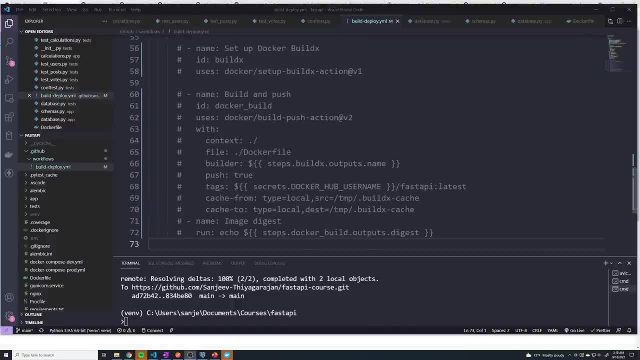 too many of our build minutes. So now that we set up the continuous integration part of our CI CD pipeline, it's now time to move on to the continuous delivery aspect of our CI CD pipeline. So this part is going to be responsible for pushing out the update to. 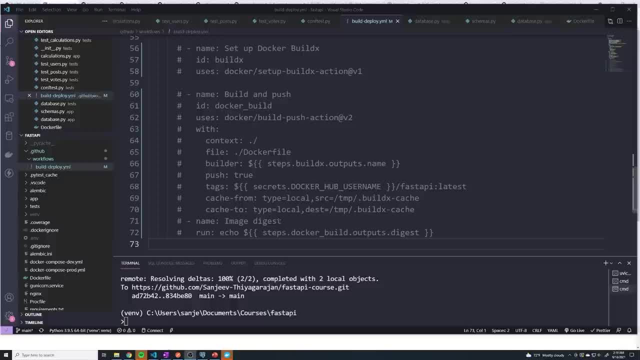 our production environment, so that our code or our production environment is running our newest and latest code. So there's a couple of things we can do, and I'm actually going to do this up here. Actually, we'll just do it down here, It's fine. So what we could. 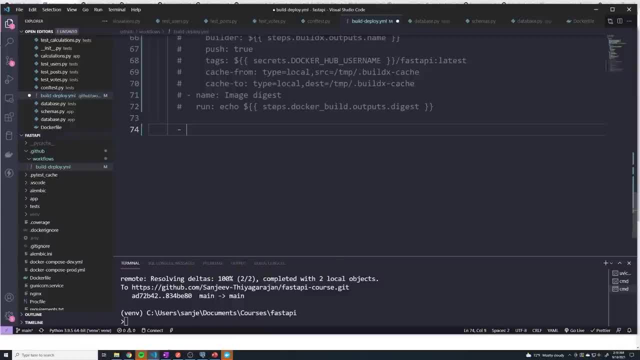 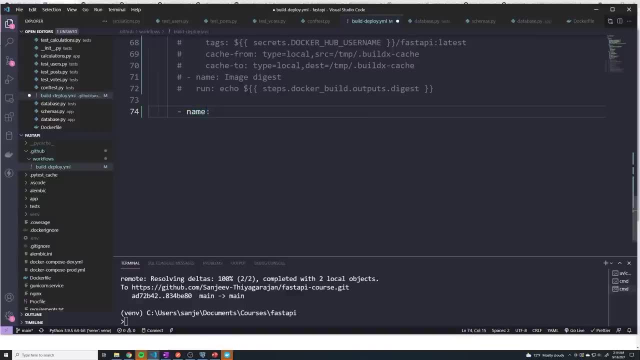 do is, you know, just to keep things simple, I could just provide another step, Right, And we can give this, you know, whatever name we want, I could say name, And then, hey, this is push changes to production, And then we can, you know, provide the steps needed. 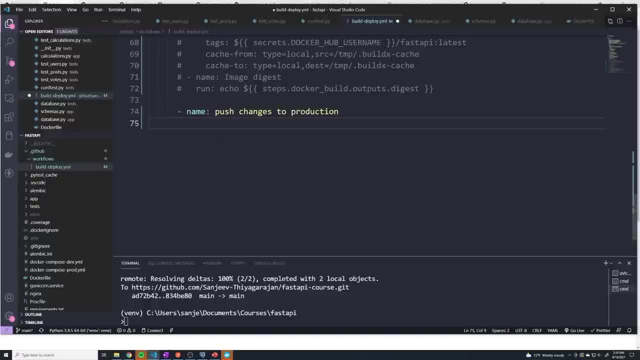 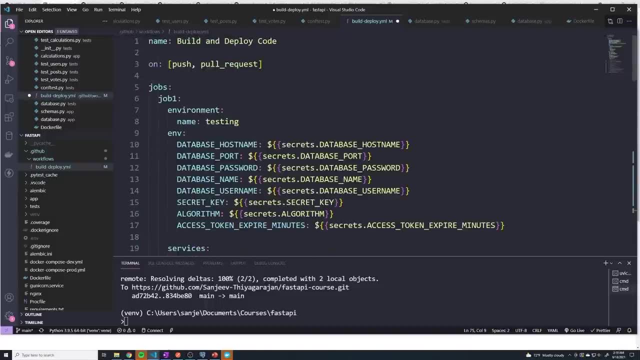 to actually push those changes Out. however, instead of doing it like this, what I would like to do is I actually want to break it out into a separate job so that we can kind of have things nice and organized, And what I actually want to do is I want to rename job one because it's not very descriptive. 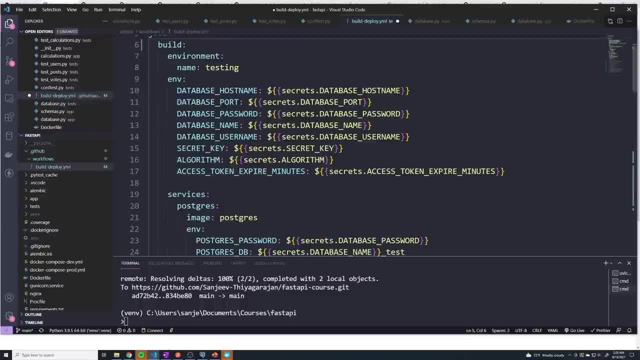 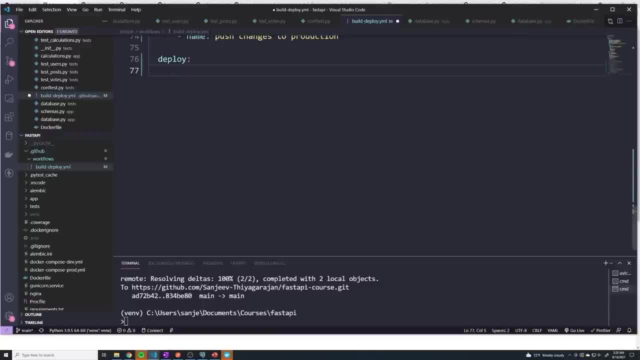 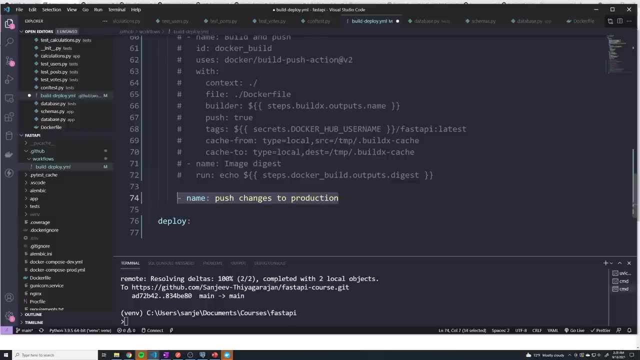 I don't know- Rename it to build, And then I'm going to create a second job and we'll call this one deploy. So we've got two different jobs. However, the the issue with jobs is that they don't behave The way that you think they would, And let me delete this. The way that jobs work is. 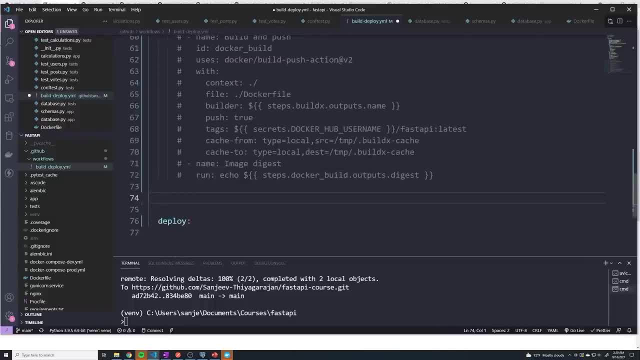 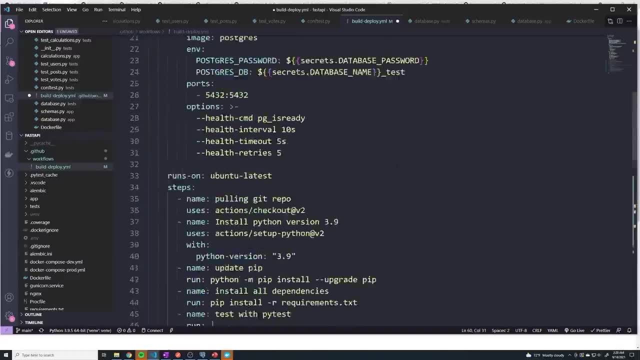 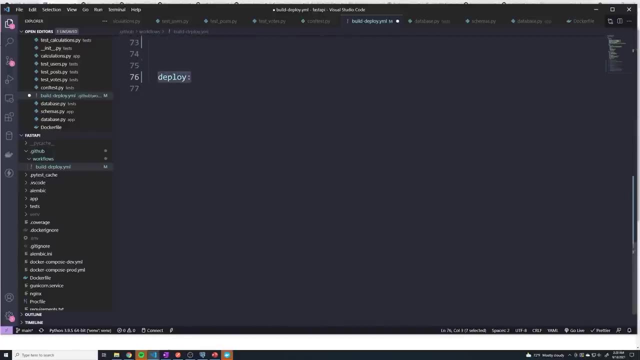 that by default in GitHub the jobs run in parallel, And so what I mean by that is that when our workflow runs, GitHub is actually going to run the build job and the deploy job in parallel at the same exact time. Now, we would definitely not want to do that, because 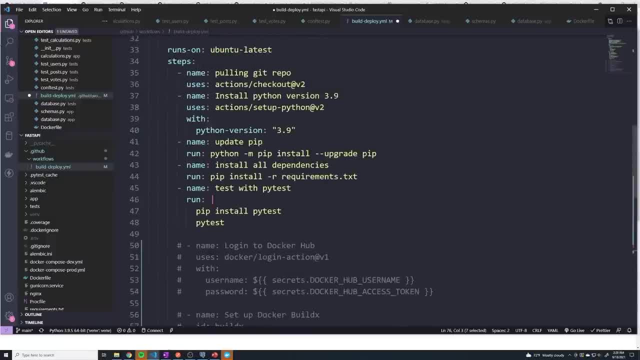 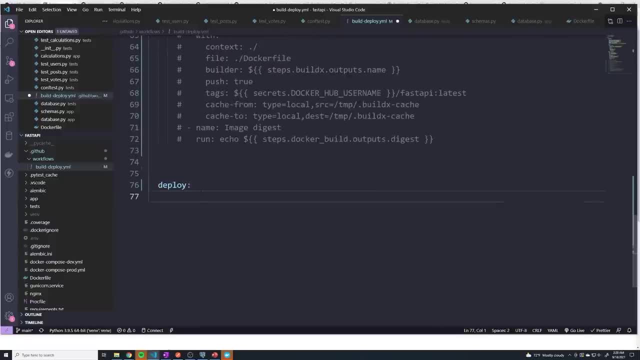 that would mean, before we've even, you know, run our tests and done anything else, we would try to actually deploy our new changes, which would be a terrible thing to happen. So we don't want it to run in parallel. How exactly do we configure that? 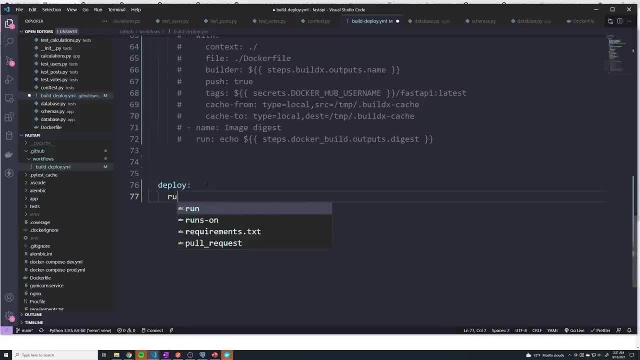 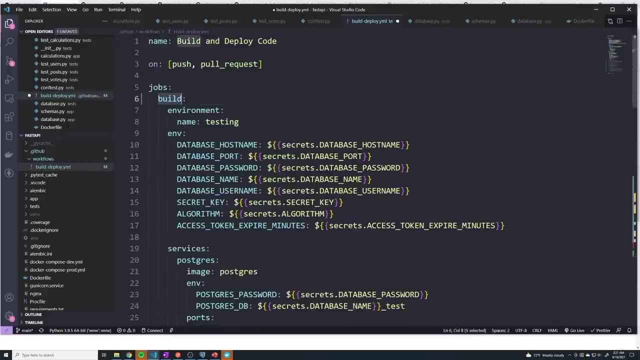 We pass in an option called runs, Sorry, needs. So you say needs And here we we tell it the list of jobs that need to complete before this job can run. So here we just say this needs to wait for the build job to run before this job runs. 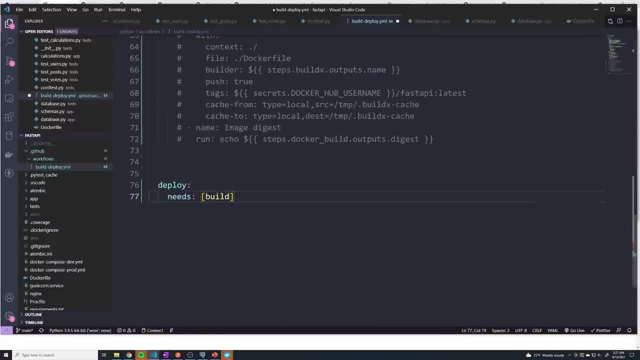 And so we just pass that into here And you could pass in multiple, multiple jobs if you wanted to. we only have one other one, So this is going to cause this to run in a sequential order And, just like with the other job, we need the runs on property to define. you know that. 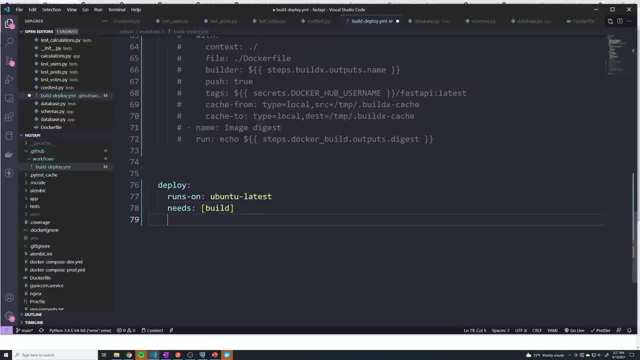 we want to run this on Ubuntu latest, And then I'm just going to create a test step. In this case, we'll do steps, And the first step is going to say uses. Actually, I'm just going to say name- you know deploying stuff- And here I'm just going to run a command. 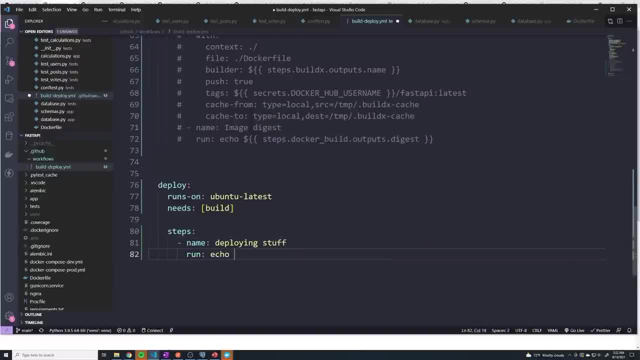 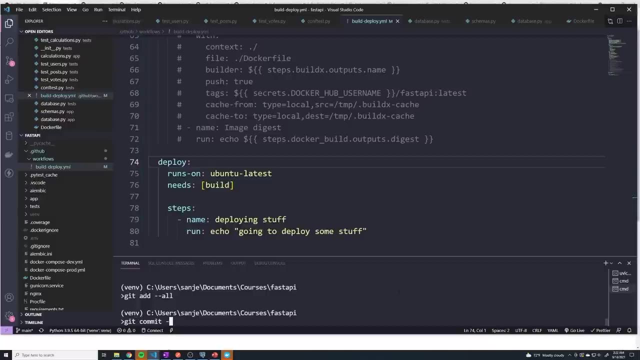 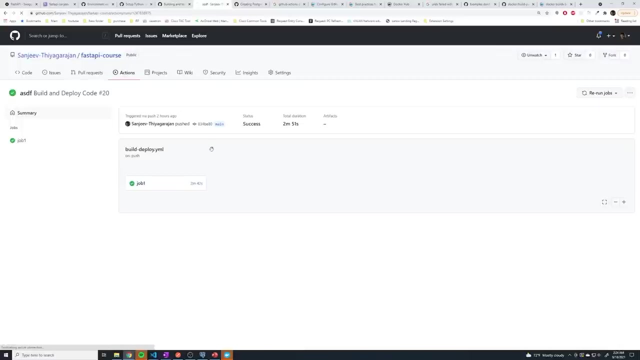 on our server And I'll just say: echo going to deploy some stuff, All right, so let's test this out. I'll do a git add dash, dash all get, commit dash m. And if we go ahead and check GitHub and go to our actions, let's take a look at what. 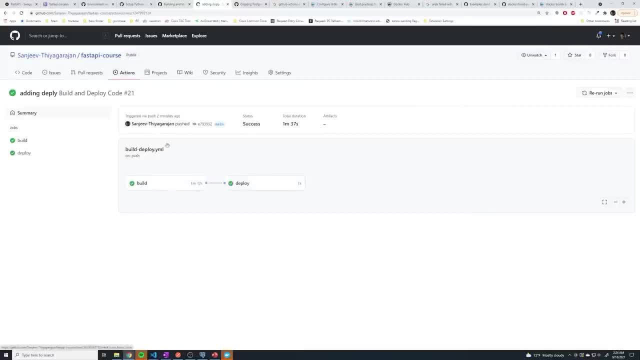 happened in the adding deploy, And so you can see now that we have two different jobs, we can actually see the two different jobs here. And so it looked like build ran just fine. And then it looked like deploy also ran just fine. And so if I take a look at 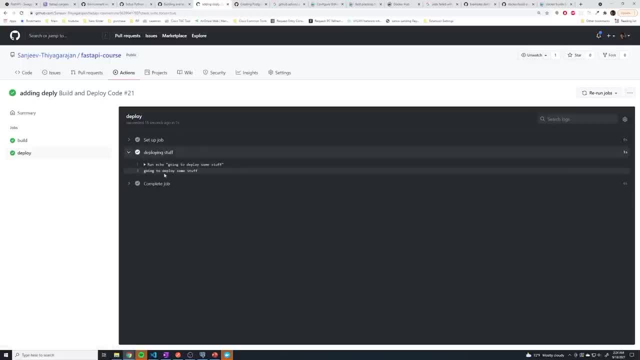 the deploying stuff, we can see that I ran the command going to deploy some stuff and it was successfully deployed, although we didn't actually deploy anything. But you get the gist of it. So now it's just a matter of figuring out what commands we need to run. 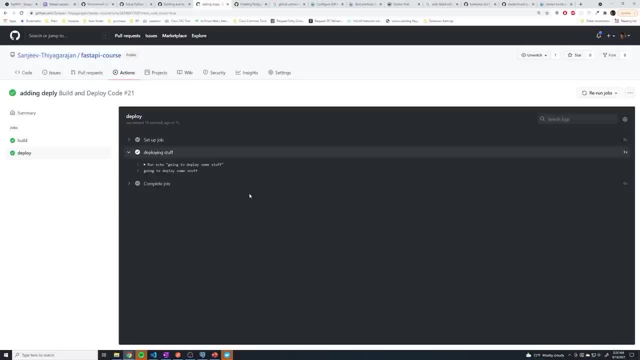 to actually push those changes out to our production server. And so you know, we covered two different deployment models in this course. there's Heroku and then there's the Ubuntu server. So we're going to start off by going over how we can actually handle this with. 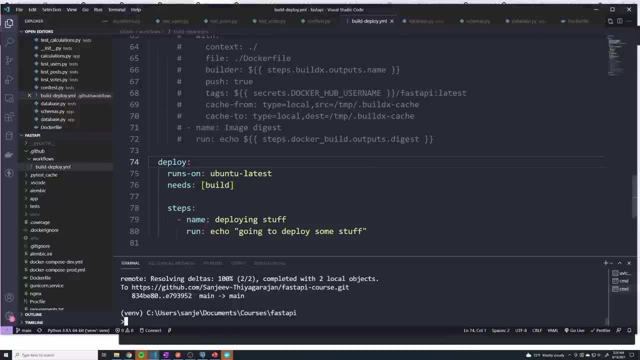 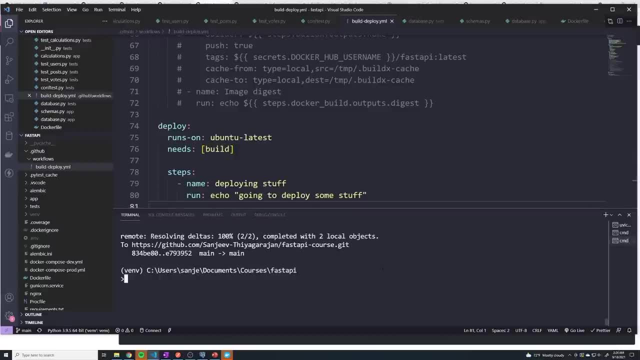 Heroku And if we go to our code right here, we're going to provide the steps to actually push an update to Heroku. Now, if you don't remember what we actually did to push changes after Heroku, do a git. 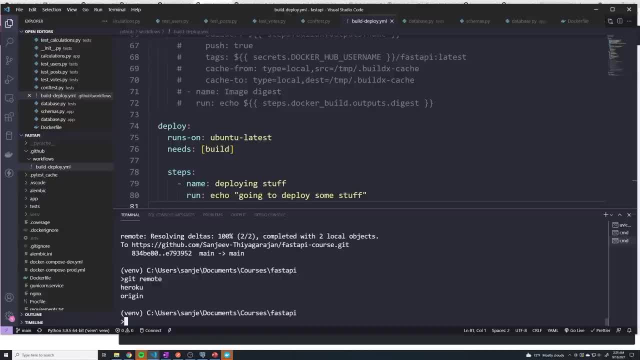 remote? I think Yep. So this is going to list out to the the Heroku remote. So if you want to actually push out the changes to your Heroku application, you would do a git push Heroku and then your branch, which is main, and that's going to update our application. 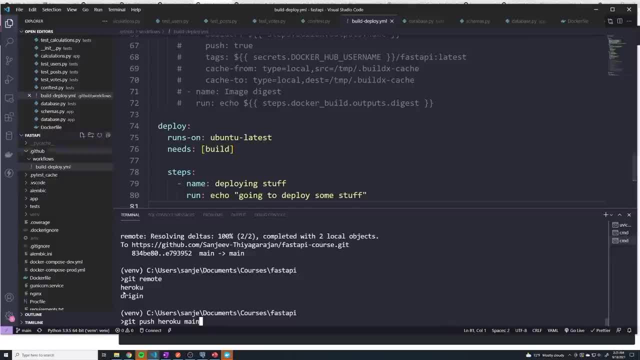 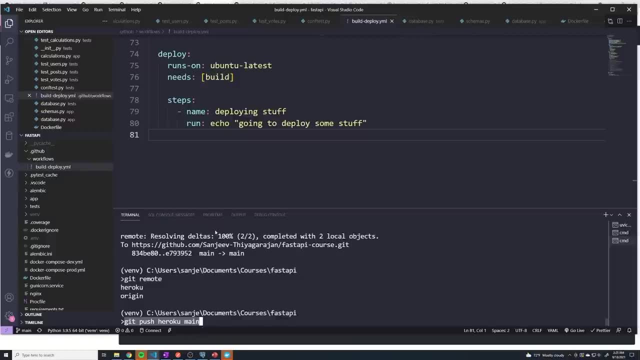 It's pretty simple with Heroku. So in this machine right in our CI CD pipeline, it's not quite as simple as running git push Heroku main. just because we don't have Heroku installed on this machine, Because when we set up Heroku we had to. 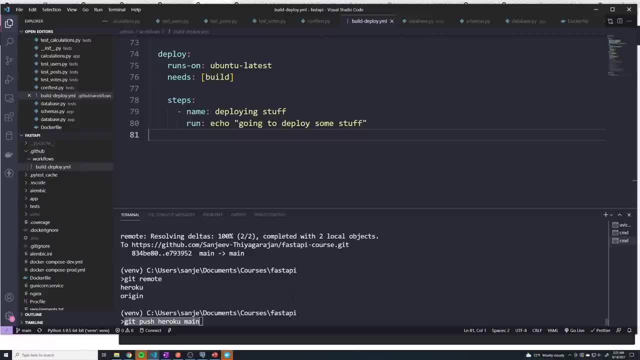 install the Heroku CLI. we had to run Heroku login, put in our credentials, and then we had to pull. we have to get our git repo, we have to add the Heroku remote and then we have to do a git push. So there's a couple of different steps And so manually doing. 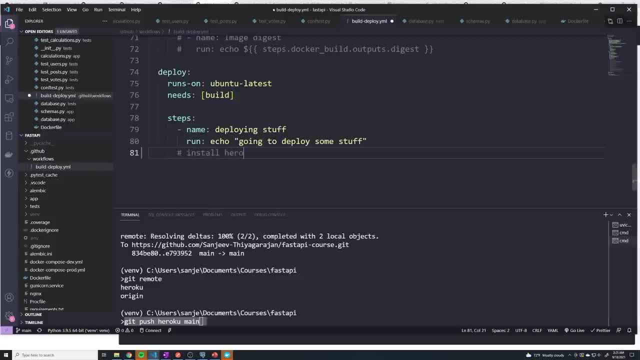 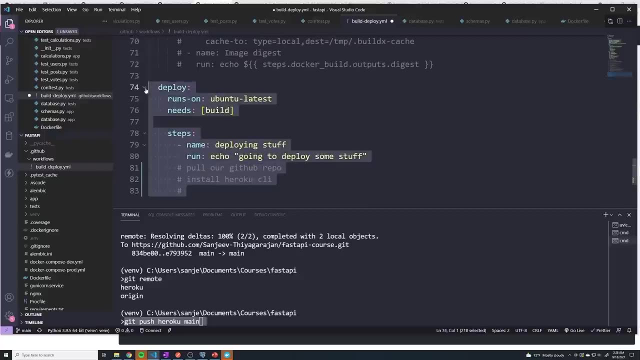 it. I just want to kind of write this out. we would, you know, install Heroku CLI. We would actually, before we even do that, we would first of all, you know, pull our GitHub repo because, remember, this job is essentially starting everything from scratch, potentially. 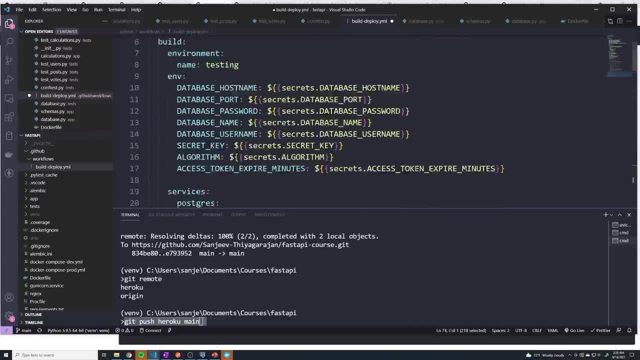 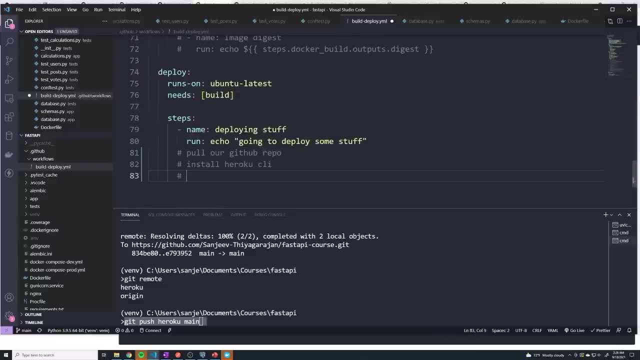 on a different machine. So anything we did here, none of this stuff is available. So we don't actually have access to the, the repo that we pulled here, So we would have to do it again here. So we pull the repo, we install Heroku CLI, then we do a Heroku login And 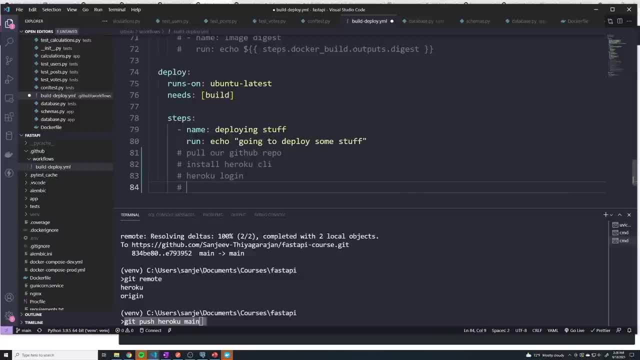 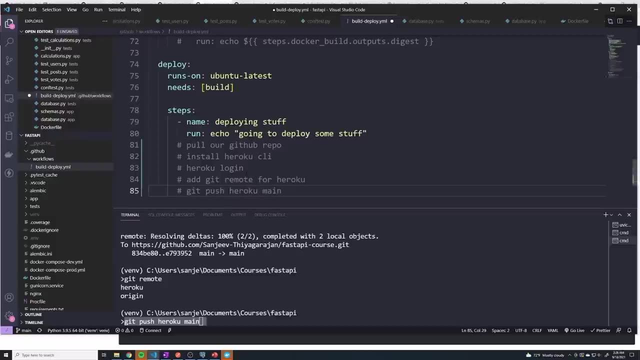 then we do a we have to add in a remote and git and I forget the command, So, but we'll just say: add git push Git remote for Heroku, And then we have to do a git push Heroku main. So those are the. 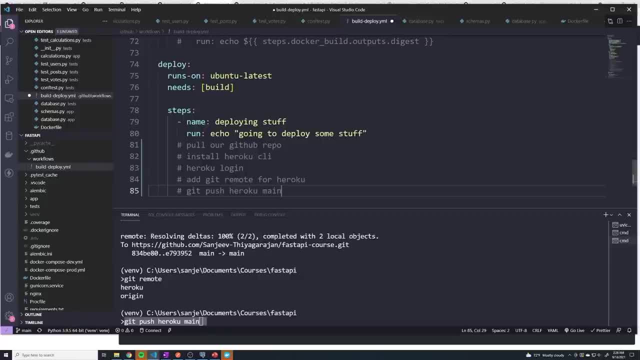 steps that we would have to run to actually deploy our application in our CI CD pipeline. And this is all technically possible. you can manually do this, But it's actually a kind of a pain in the butt to actually do this And instead what I recommend you do. 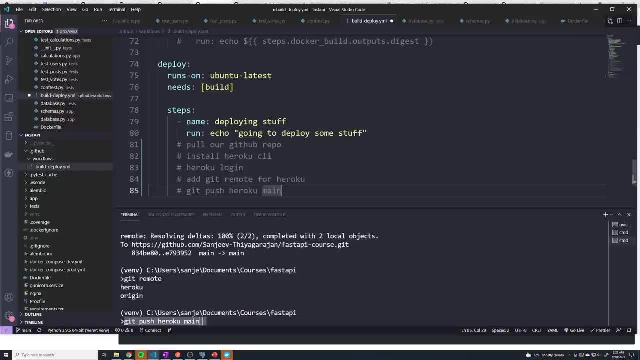 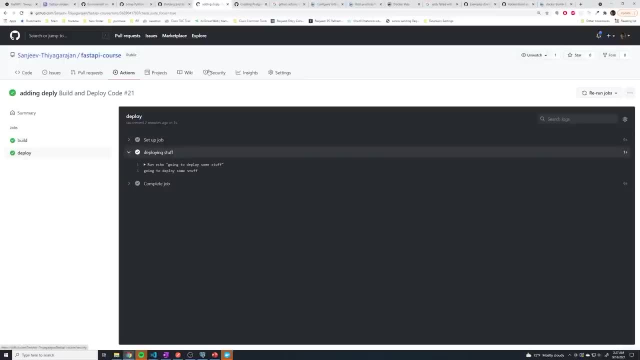 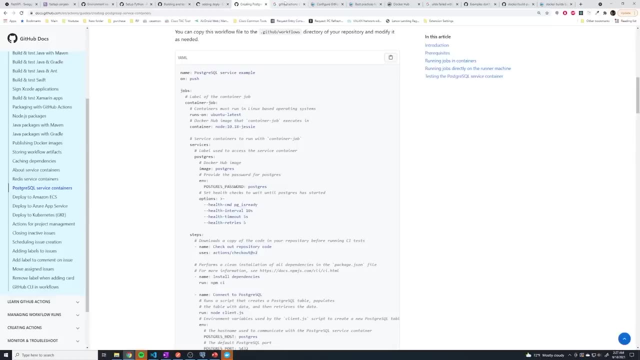 is look for a, a action in the GitHub marketplace that kind of does this all under the hood. So that's what we're going to do Because, you know, deploying to Heroku is a very common task. So if I go to the marketplace, which I forget which tab was the marketplace? Oh, I think. 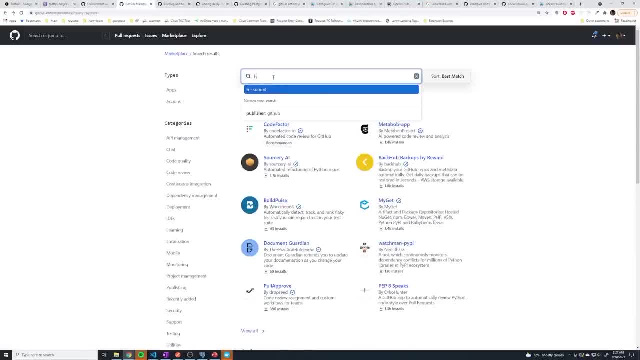 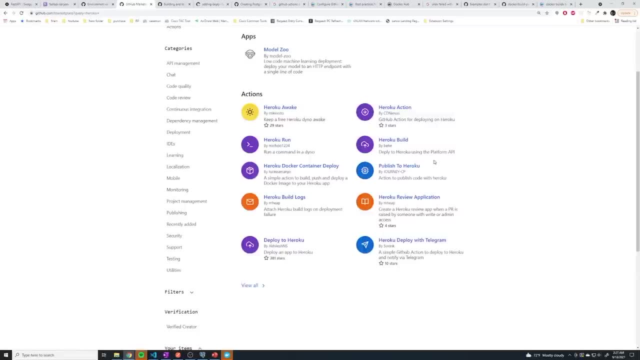 it's this one, Yeah, And so here, if I search for Heroku, you'll see that we have a couple of different options for deploying to Heroku in the marketplace. Let me just see view all, because I got to figure out which one is the one that I want And this is the one that. 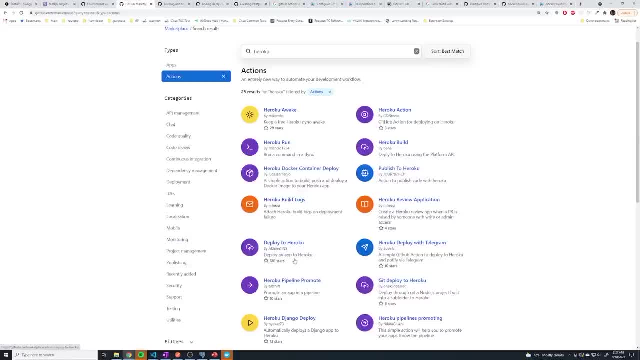 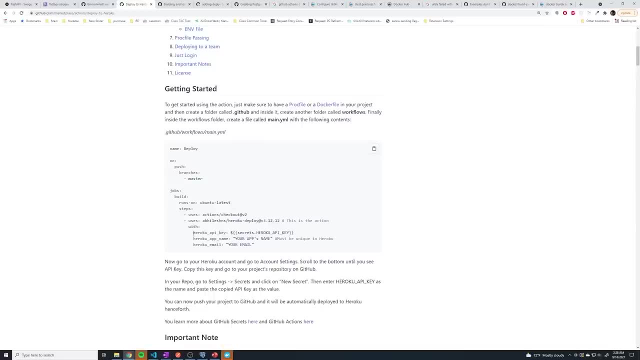 I want by Akilesh NS. So this is the one that's got the most stars, So we'll select this one, And you'll see that in the example. the way that we actually deploy to Heroku is: we have to get a Heroku API key, we have to provide our Heroku app name and then we have to provide. 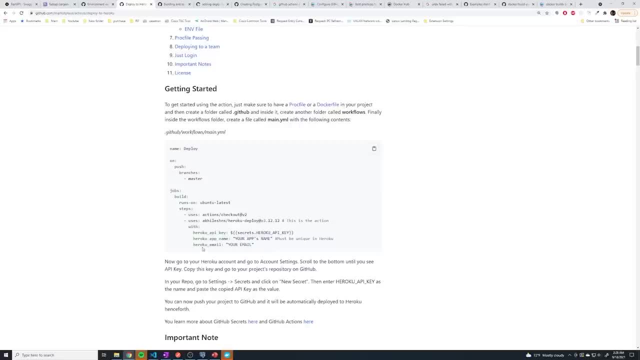 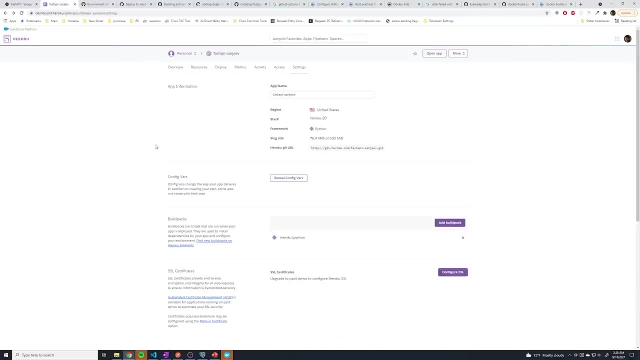 our Heroku email. So let's get this from our account And then we will create secrets within our GitHub repository So we can store the information, because we don't want to hard code that into our YAML file. So, going back to Heroku, if you go to your account, which 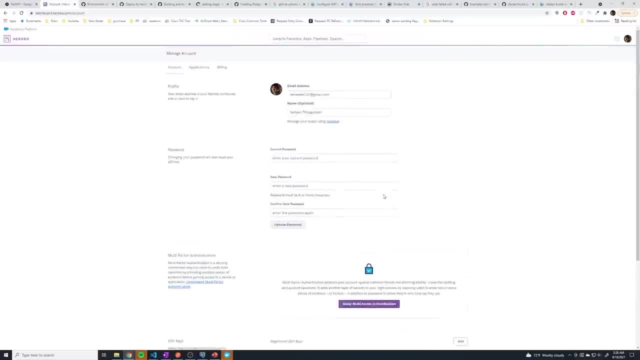 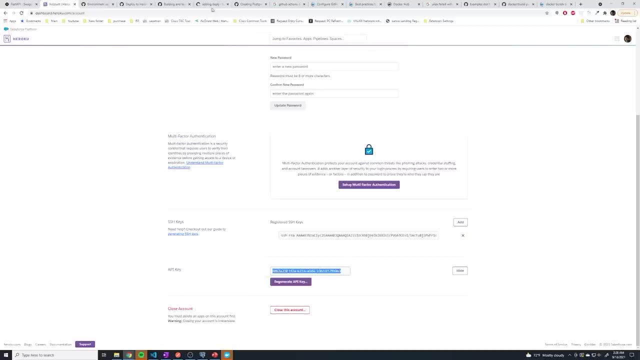 is the little logo here- then select account settings. you'll see that the API key is right here, So we can just like reveal, And then I'm just going to copy this key And what we're gonna do is we're going to go to our GitHub repository, we'll go to settings And 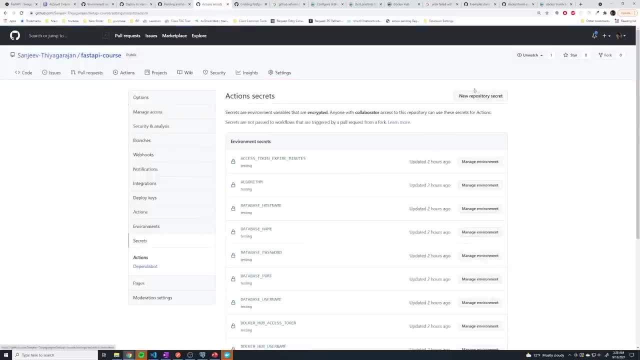 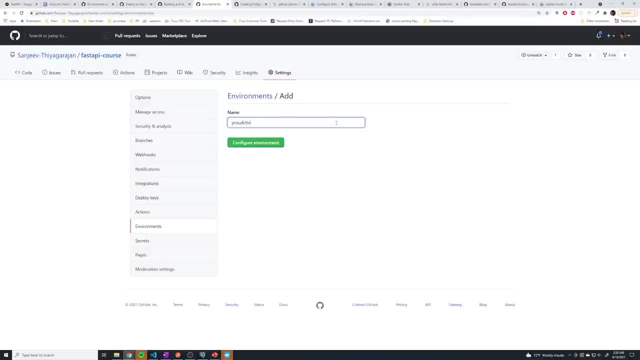 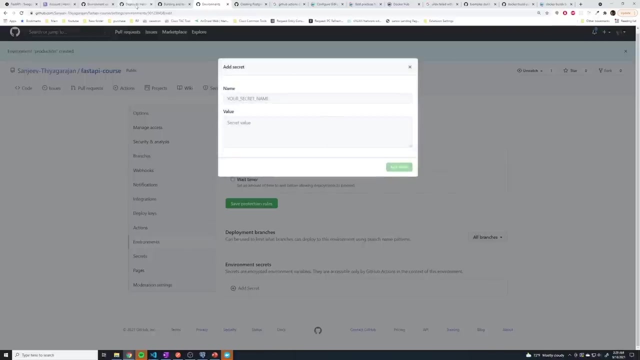 then we can create our secret, So you can create a global repository secret, or you can do what I'm going to do, which is I'm going to create a brand new environment for production. we'll call this production- That is not how you spell production- And we're going to add a secret And I'm going 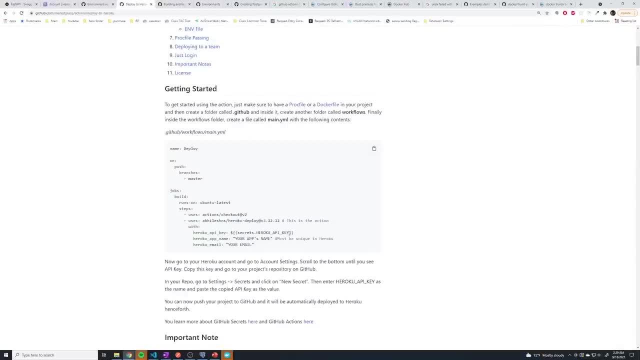 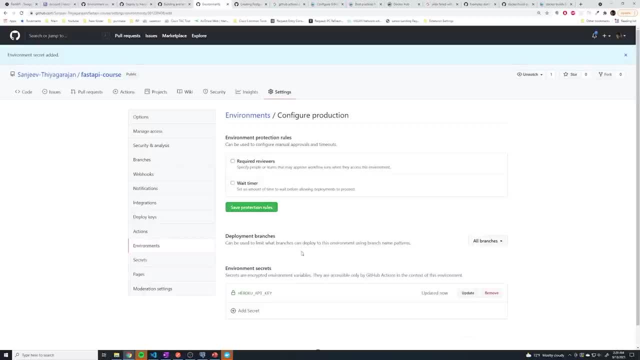 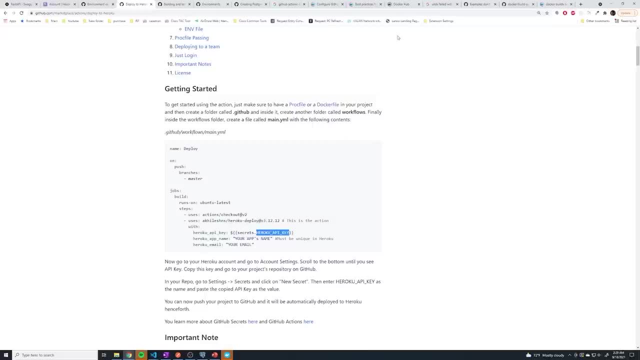 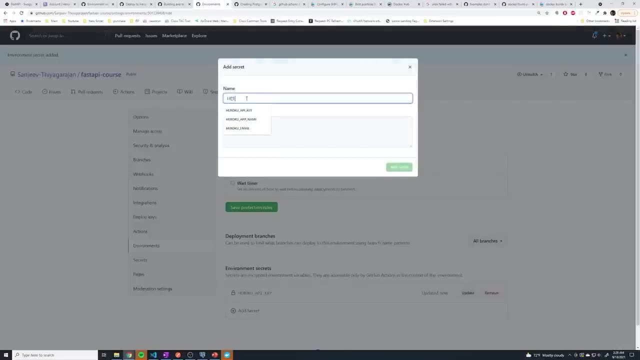 So Heroku underscore API key, Add secret. And then what else do we need? we have to add the email. So let's create a secret for the email as well, because- why not? they didn't do that, but we're going to be a little bit more secure And I'll call this Heroku underscore. 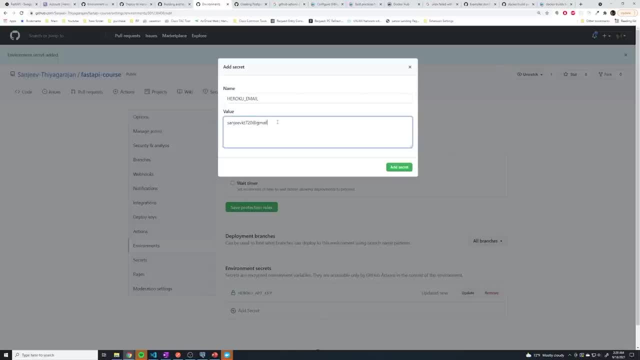 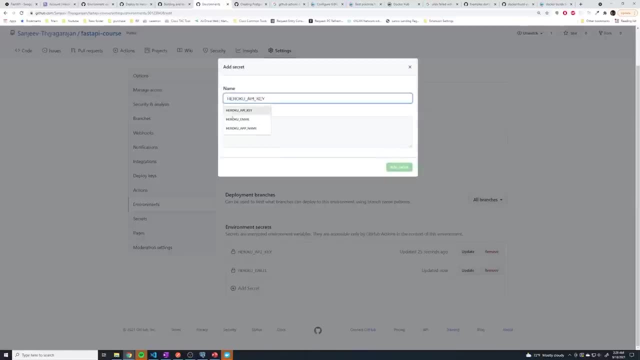 email- And this is just going to be your email- that you used to register, Is that? And then, if you want to, you can also add the Heroku app name as a secret as well. You don't have to do this, but I'm going to do it. 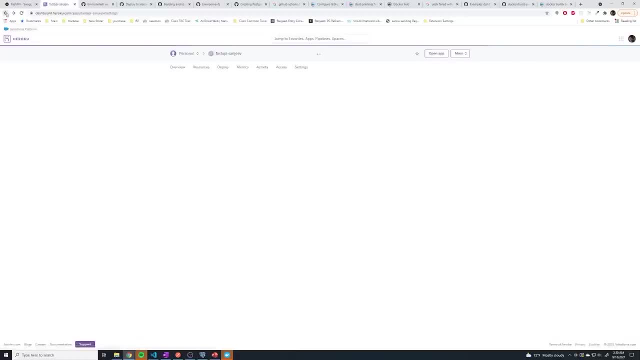 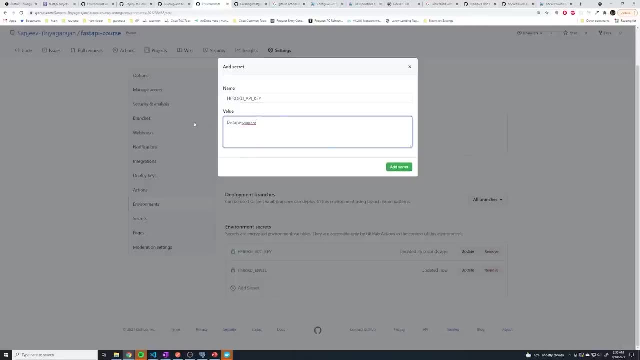 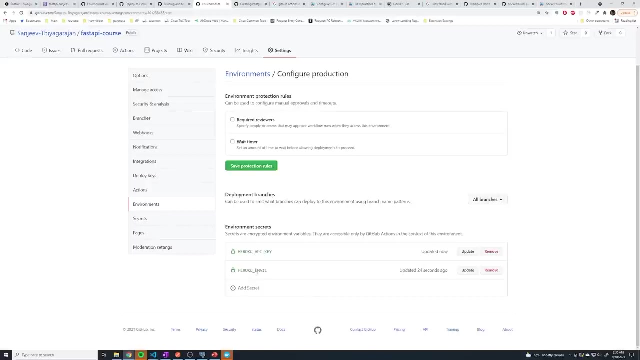 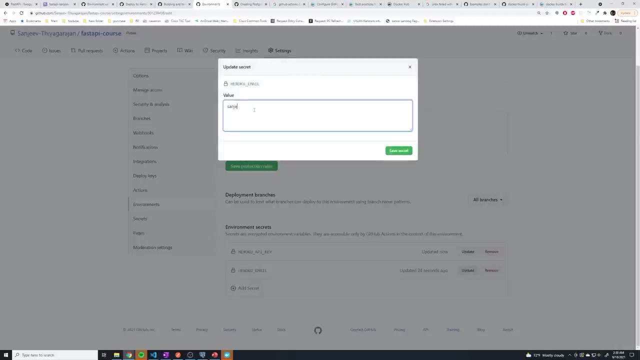 And what did I call my app? I can't even remember Fast API. Sanjeev, Yours is going to be different, so make sure you update it accordingly. Okay, so wait, what happened here? Why is there only two? I think I may have accidentally overridden one of these keys. 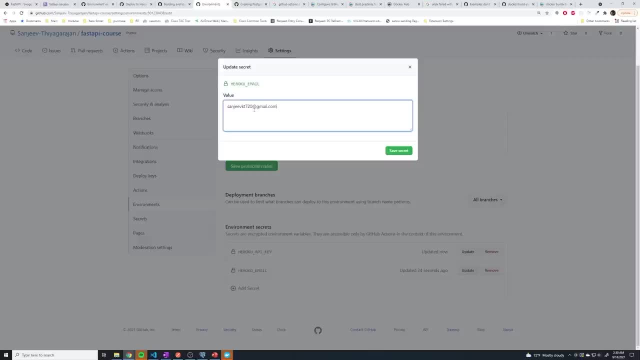 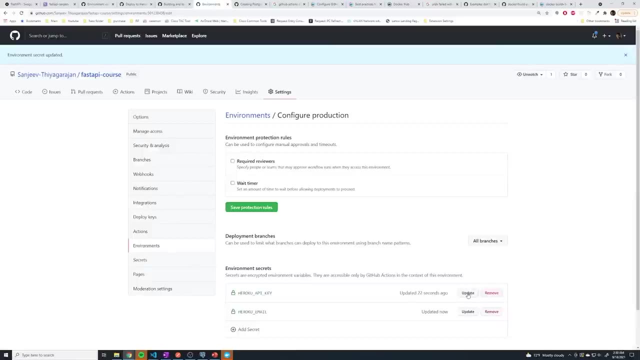 So let me put this information back in just in case, because you can't actually look at the keys after you save them. You can only update them. Okay, so we updated that and then the API key. I have to copy this once more. 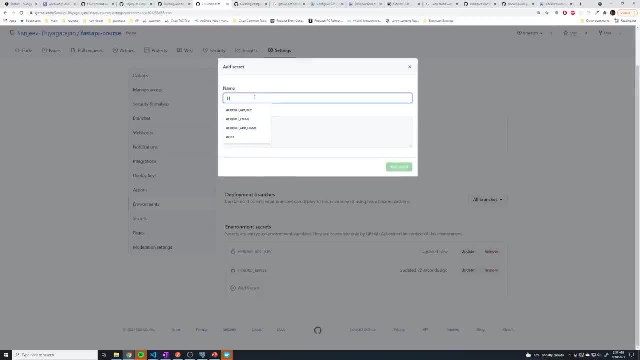 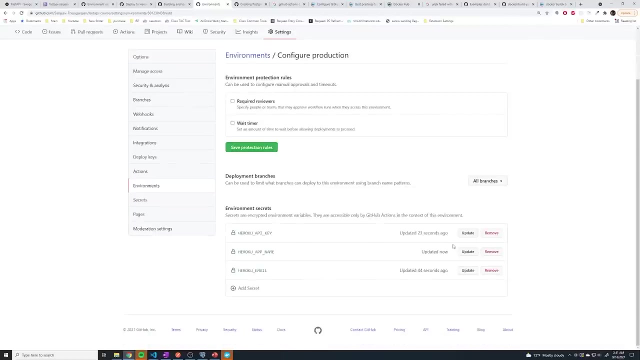 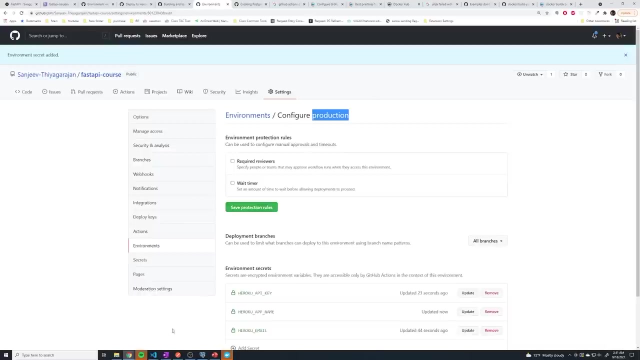 All right, so we've got those. and then let me once again add the Heroku app name. This is going to be All right, so now we've got our three keys. Hopefully I set those all up correctly And keep in mind the name of this environment is called production. 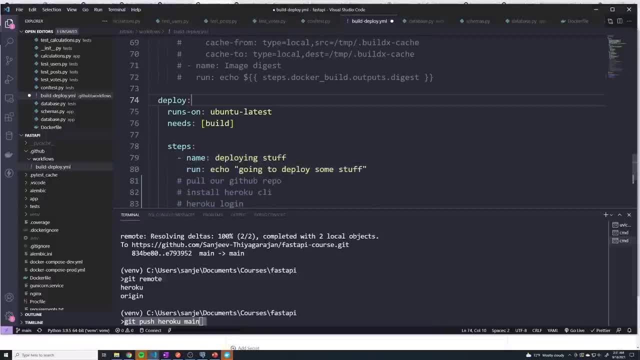 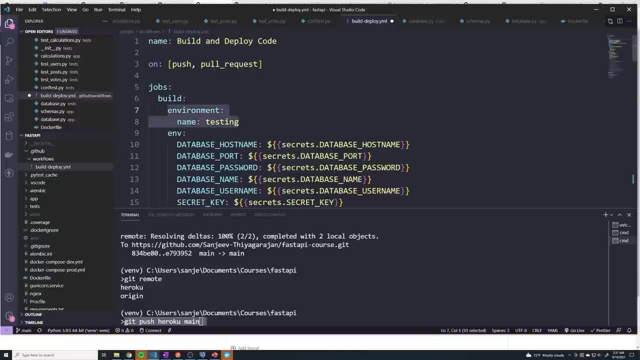 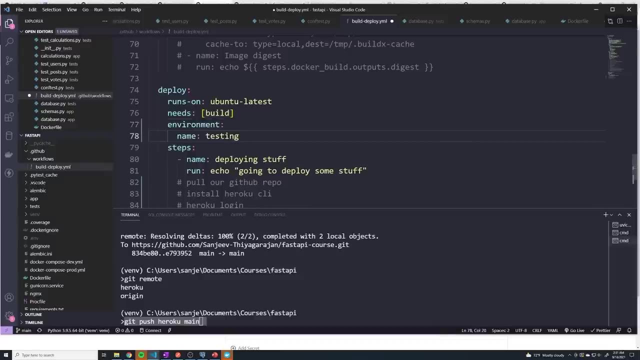 So for the other job, which is the deploy job, we're going to specify the environment just the same way we did with the first job, just by referencing This, This code, right here, and just updating the name, And so this is going to be production. 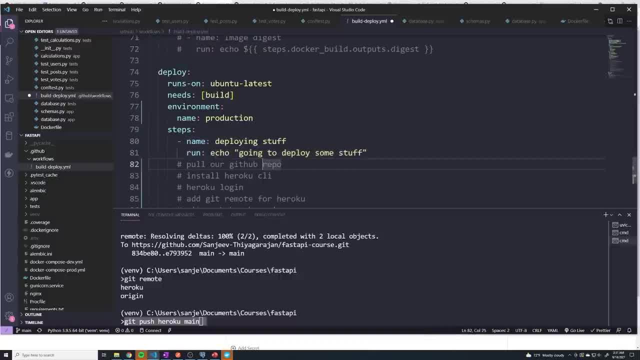 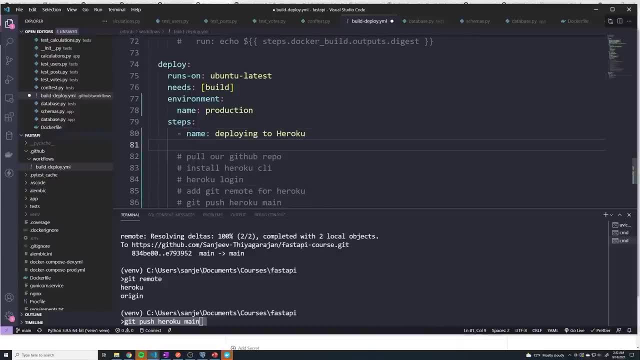 And then we can remove this unnecessary step And actually I'll change this to be deploying to Heroku, And then we'll change this to be use, And so, just like in the documentation- actually I might as well just copy it- 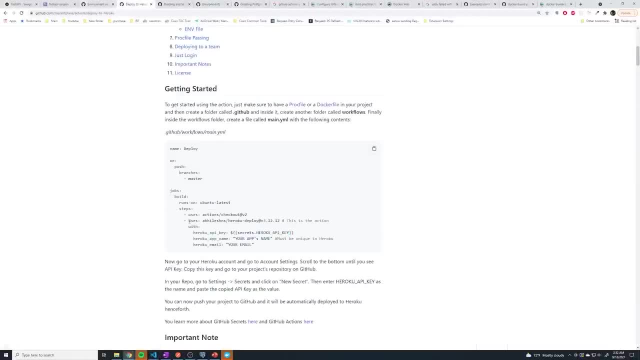 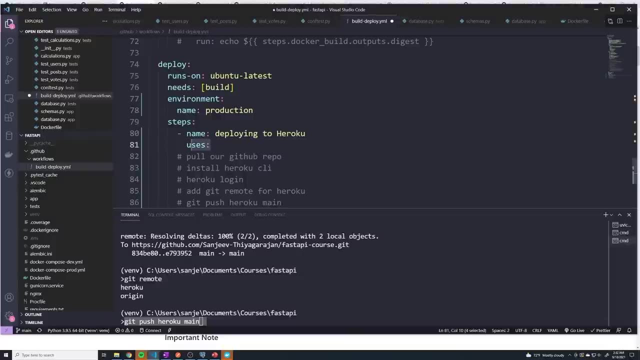 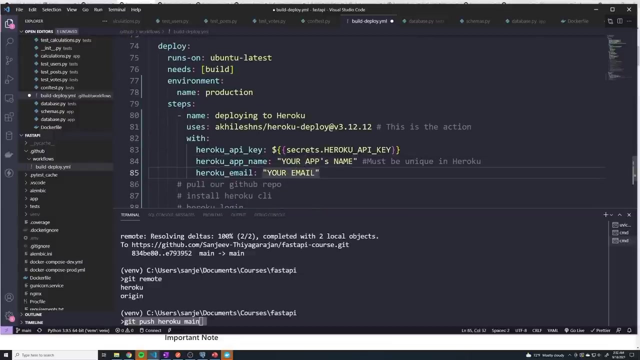 because it's going to be used, Because it's a little bit easier, So I can just copy this And we can just update the app name with the secret that we defined: And, And, And e-mail, As well as the secret for the e-mail. 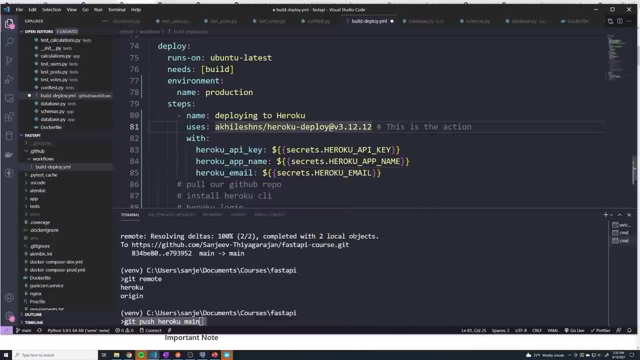 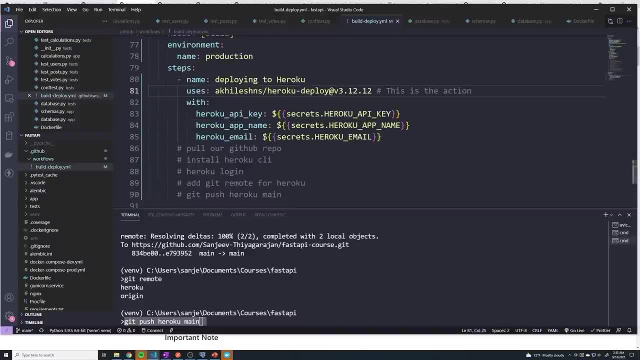 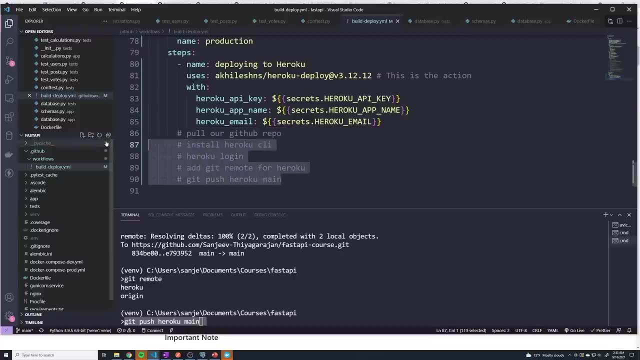 And that's all we have to do. for the Heroku side of things, We don't. It's as simple as that. So that's why I always recommend you look for a built-in action, so that you don't have to perform all of these steps by yourself. 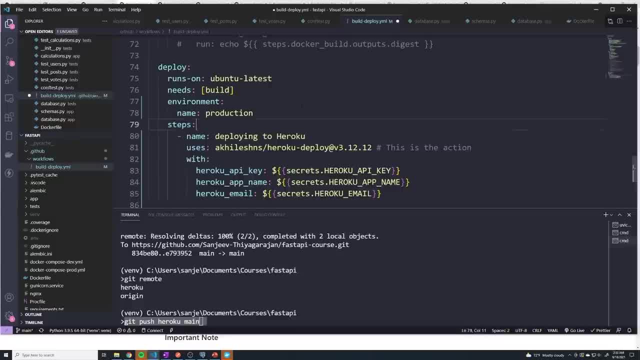 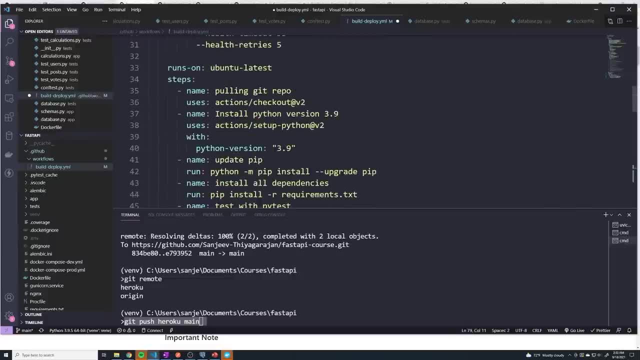 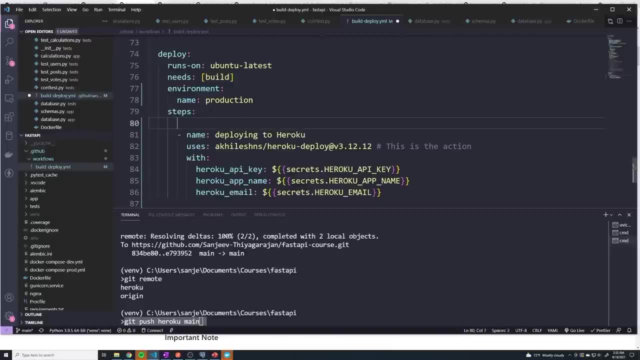 And I realized before we even do that we have to actually pull our code, just like we did in the first job. So we're going to copy that section right here where we pull the repo. All right, so we've got the repo and then we deploy to Heroku. 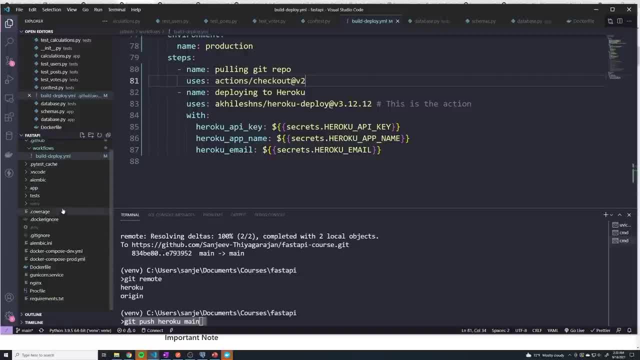 And so what I'm going to do now is we want to check our code real quick and make some changes. that'll be easy to kind of quickly just test and see that we actually pushed out our changes So under our mainpy file. you know, I'm just going to do what I always do. 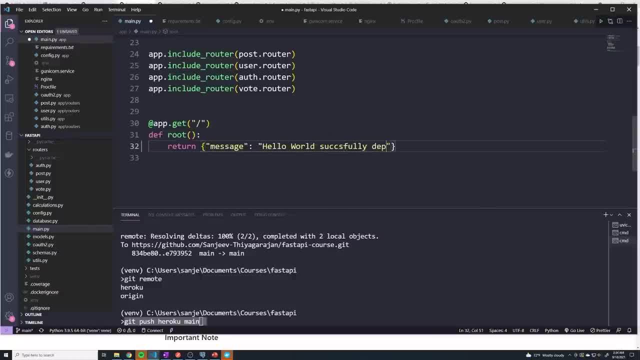 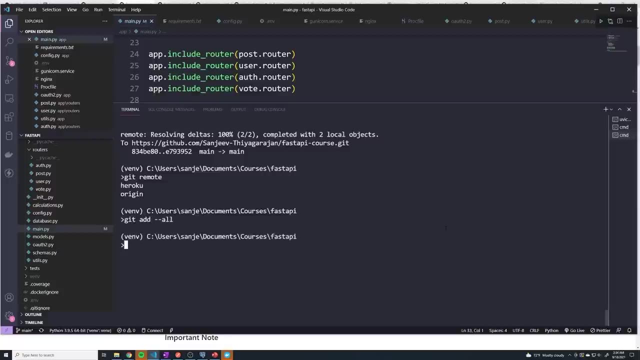 I'm just going to add: successfully deployed from CI CD pipeline okay, And so going to save that. and then now we want to do a git add dash, dash, all git, commit dash m Push to Heroku example. and then we'll do a git push origin main. 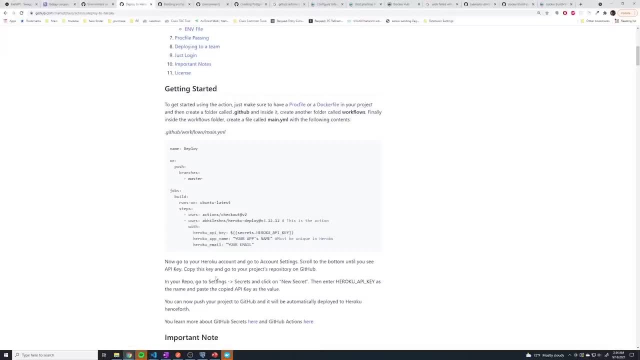 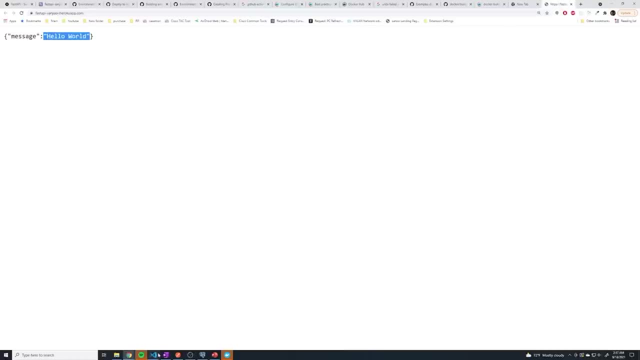 And before I do that, let me go to my app. So if I actually go to my app on Heroku, we can see it just says message: hello world. And so after we commit these changes, we should see it send the new message message. 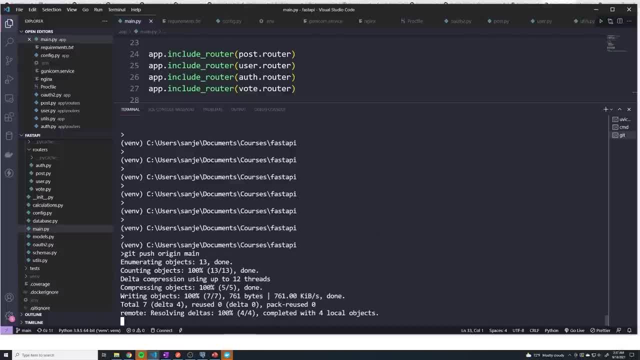 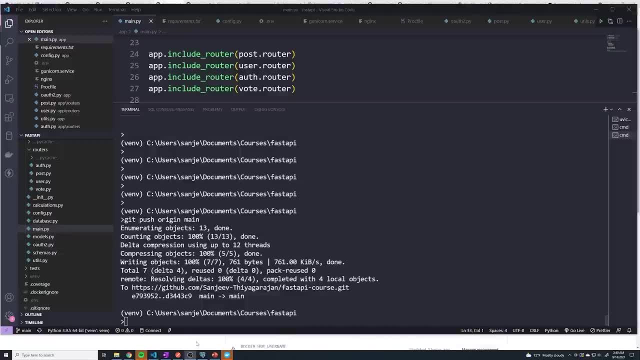 So I'm going to send a push this to GitHub now and our CI CD pipeline should run and push those changes. All right. so now if I go back to GitHub and we take a look at the actions, I can see my push to Heroku example succeeded. 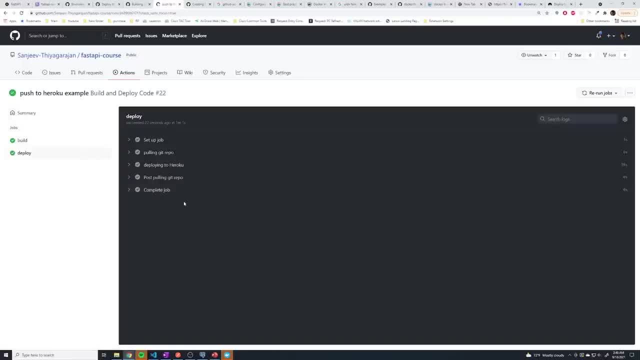 And so you can see both the build phase and the deploy phase both succeeded. And if we want to take a look at the notes and then just see what happened with the deploying to Heroku section, we'll see the logs for this specific step. 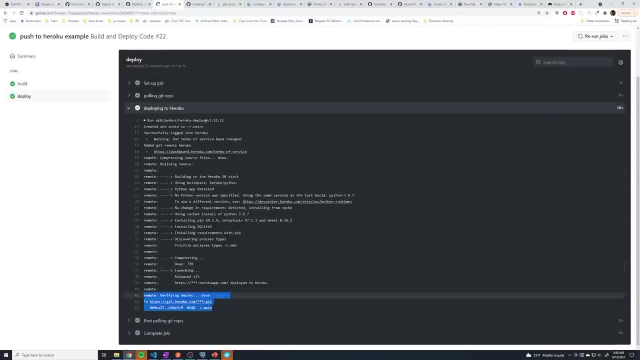 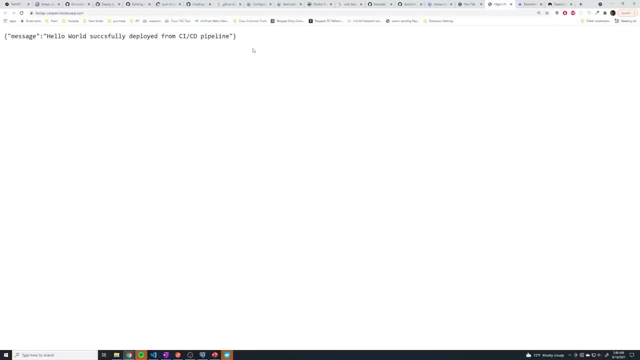 And so it looks like we can see Heroku is running in this case and it looks like everything worked. So if I go back to my app and hit refresh Right, we could see we get the new message. So we have successfully updated Heroku using our CI CD pipeline. 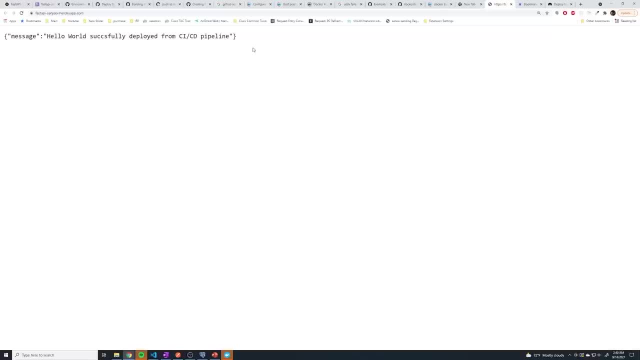 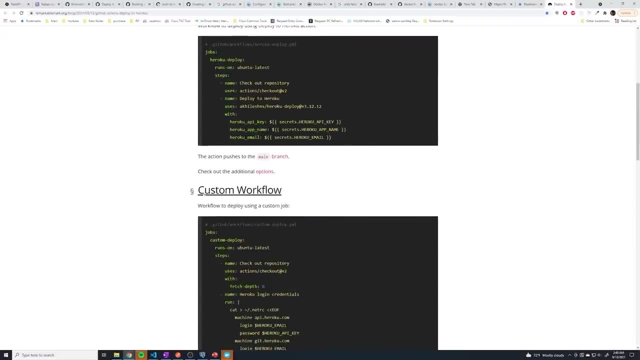 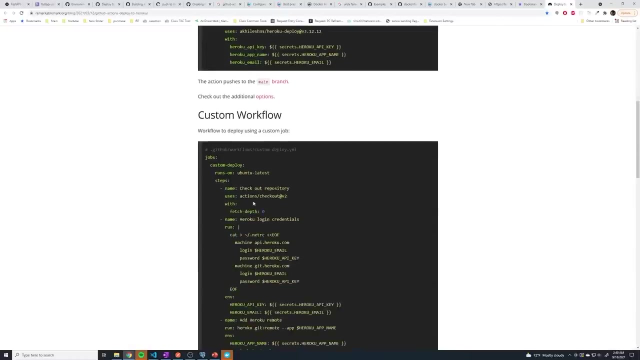 It's as simple as that. And before I wrap up this video, this section or this video on deploying to Heroku, I found this one good article that shows you how to deploy to Heroku in a manual way. So if you don't want to use the built in or the pre configured GitHub action, you can. 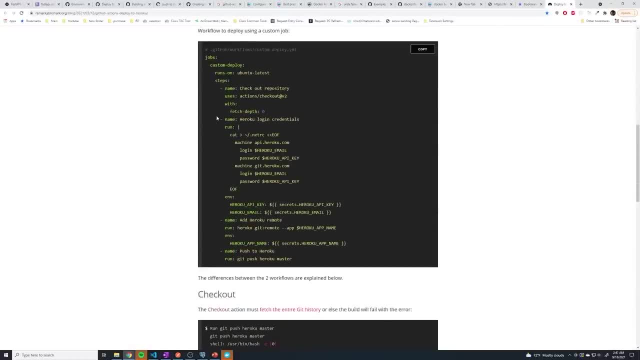 actually create a custom workflow when it comes to, you know, actually manually logging. So if you don't want to use the built in or the pre configured GitHub action, you can actually create a custom workflow when it comes to, you know, actually manually logging. 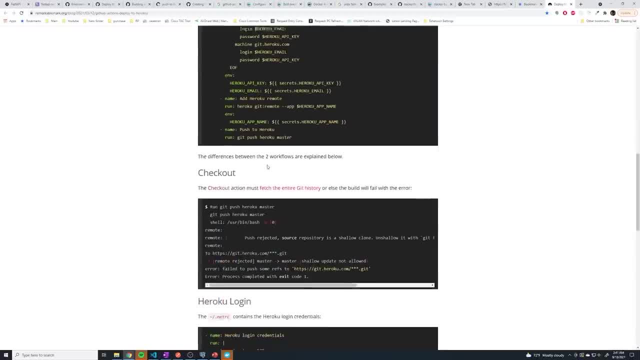 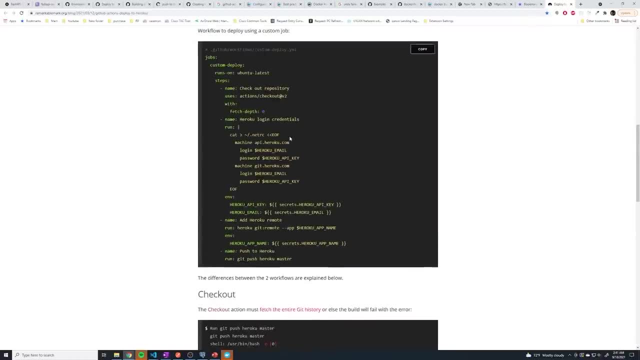 And then pushing all of these changes out to Heroku the manual way instead of using that pre built action. But this is a little bit more complex And this would only really be needed under very specific circumstances or just for learning. or just for learning purposes. 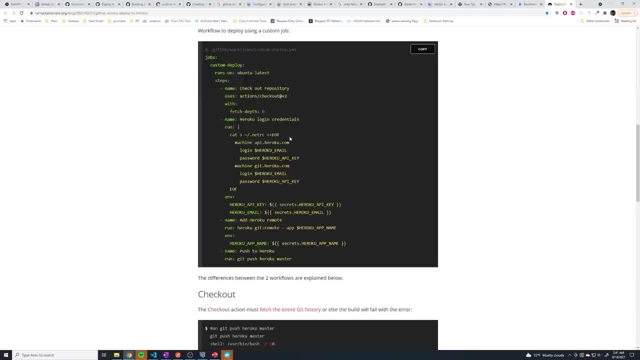 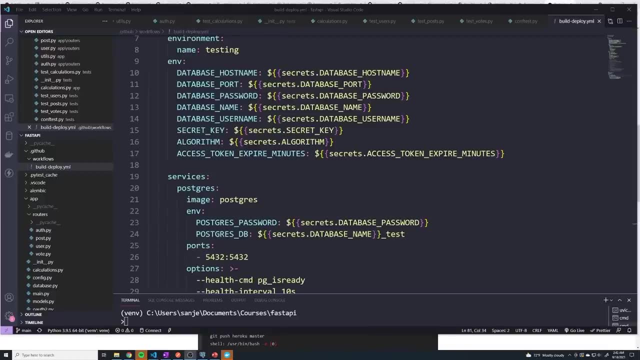 So take a look at it if you want to see how it's done manually, but you never actually have to do that. Now, before we move any further, there's one thing that I want to check to make sure that our CI CD pipeline properly does. 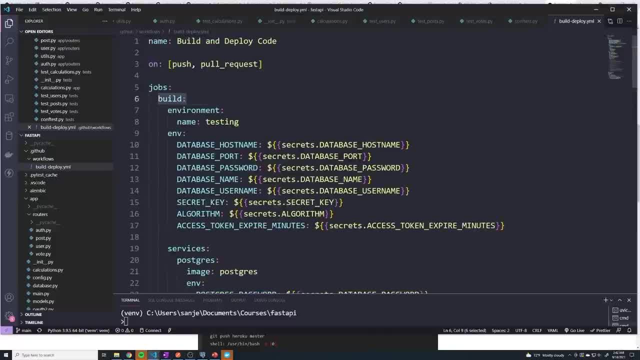 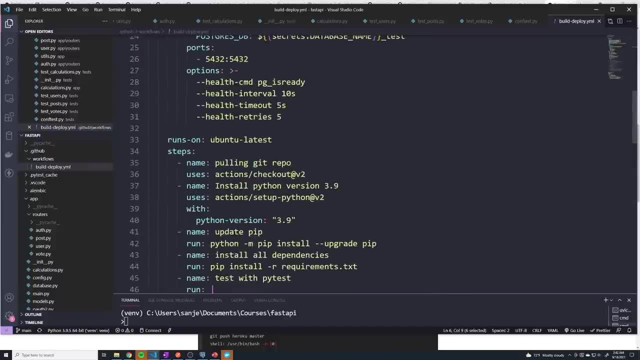 And that is that If we get any kind of errors in the build job, I want to make sure that the deploy job does not run right, And so when I say errors, it could be anything right. maybe we're unable to install all of. 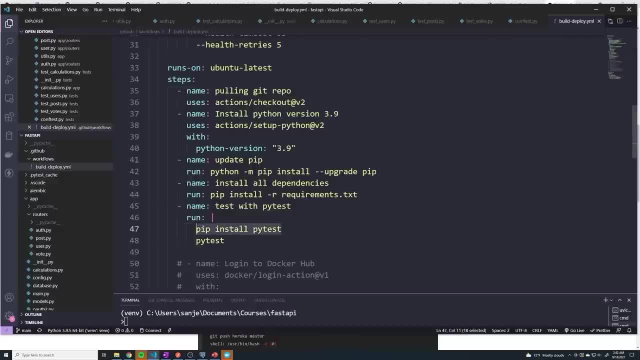 our dependencies or maybe, and more importantly, if our tests fail. right, if my tests fail, I don't want to push my broken code out to production. So I want to make sure that if the test fails, we stop right there and we don't proceed. 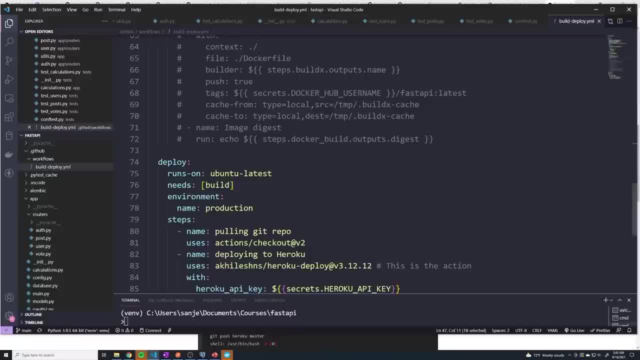 any further with the deploy, And so from a configuration perspective, you don't technically have to do anything. that's the default configuration, But I do want to verify that it actually does what we expect it to. So in the tests files, if I can find it tests, I'm going to go to. you know, it doesn't really. 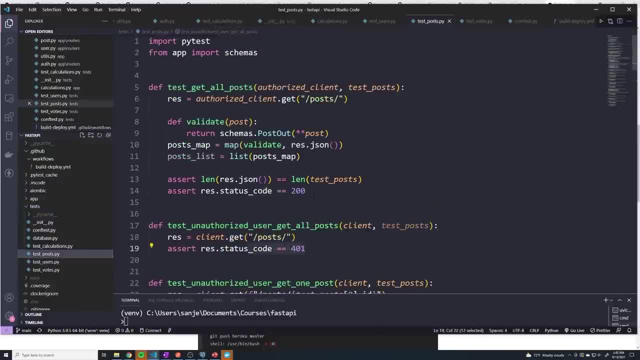 matter what test, I'm just going to go on to test posts And I'm just going to modify this to an incorrect value. I'm going to put this in the notes change to this one, So I remember which one I changed, so I can change it back from 200. 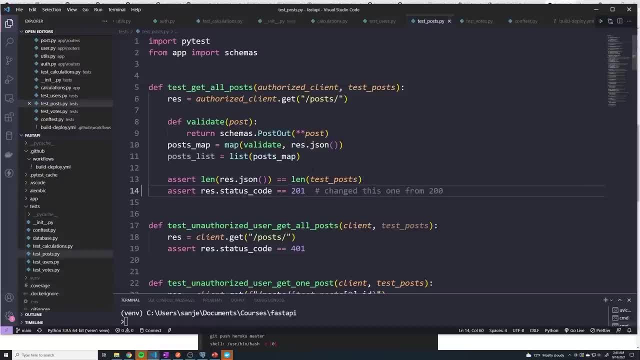 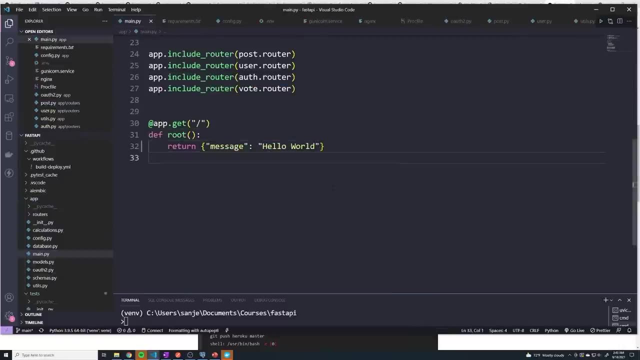 So this should cause this test to fail. And if the test fails, then we want to make sure that we don't deploy- And I'm also going to go back to our main dot p y file to actually make some visible changes by changing this back to Hello world to see if our code actually got updated accidentally. 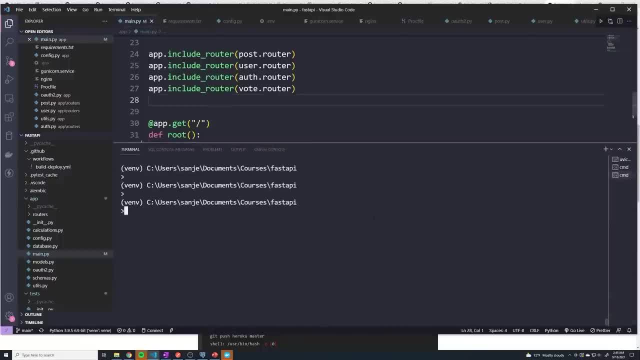 or not. So we got everything set. We'll do a git add once again, We'll do a git commit dash m Broke stuff And then we'll do a git or git push origin main And we'll let that run. 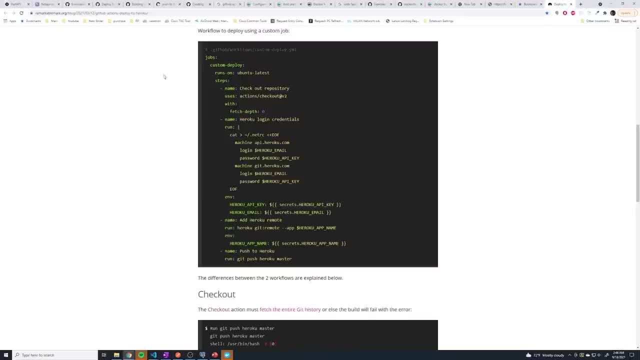 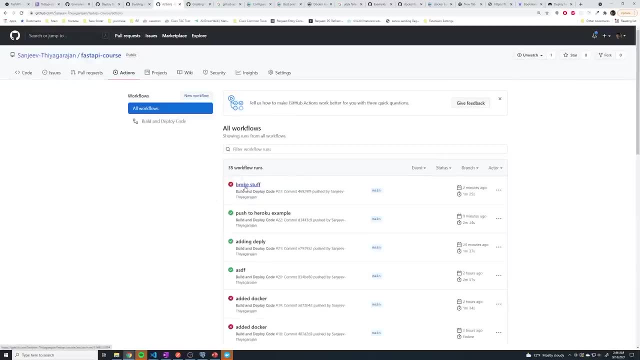 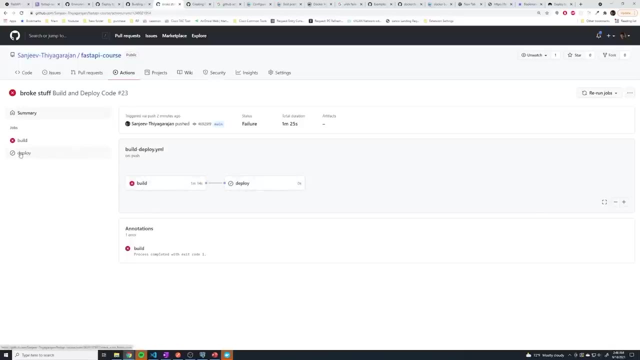 Alright, so going back to GitHub now let me go back to these, the Actions page, And we can see the last run. it looks like it failed. So let's see where it failed And so you could see here. it failed in the build stage and then the deploy stage. I 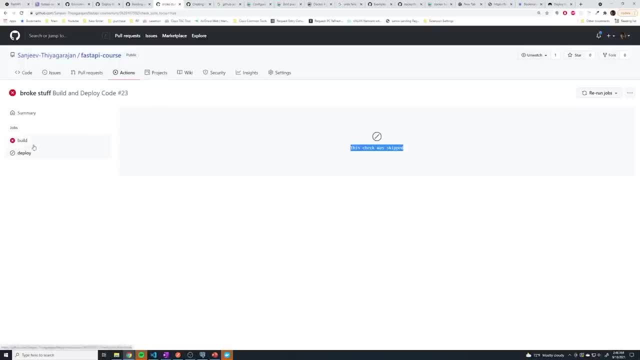 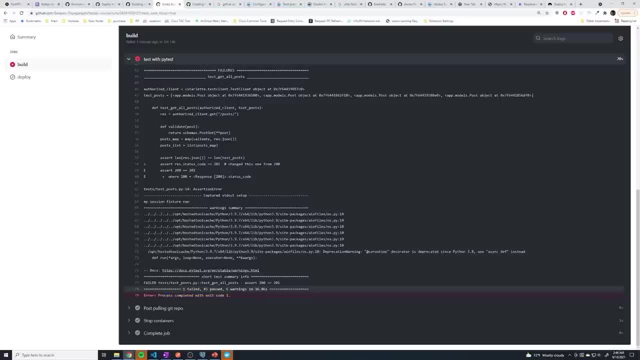 checked this. this check was skipped, So that means we actually did properly skip the deploy phase because the build phase failed, And we can see that we exited with an error code because one of our tests failed. Awesome, So let's go back. 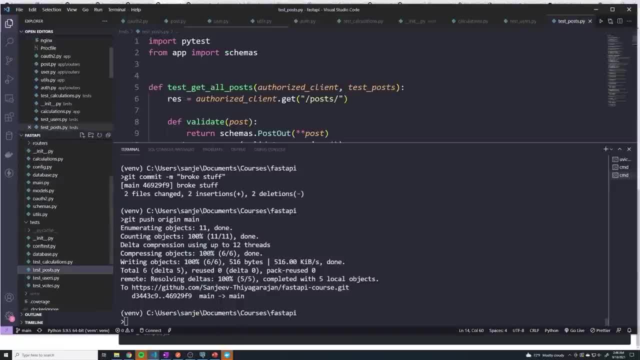 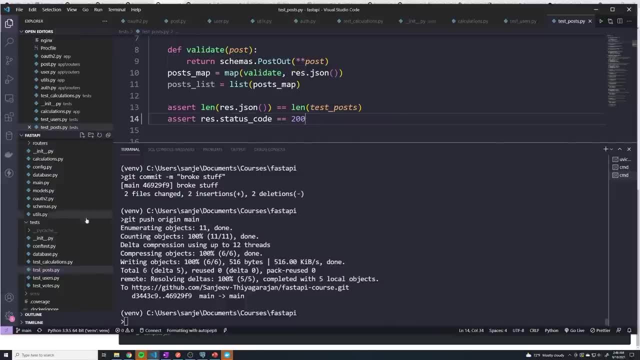 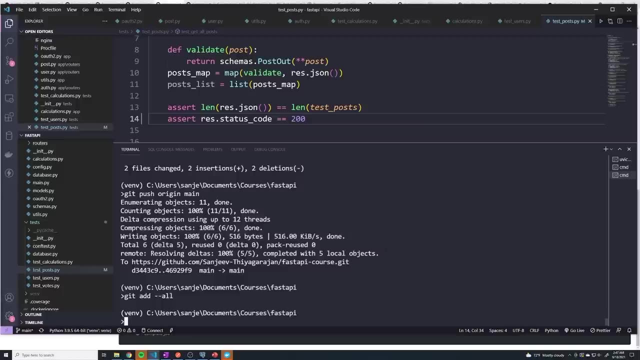 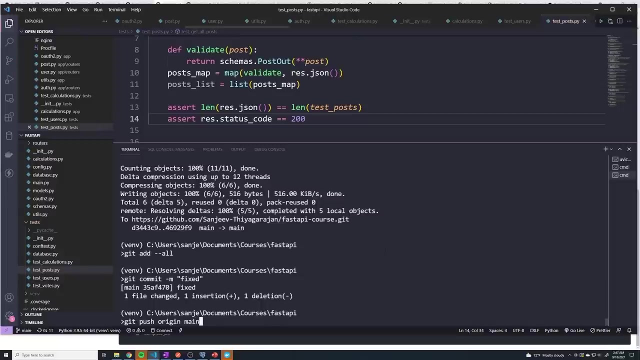 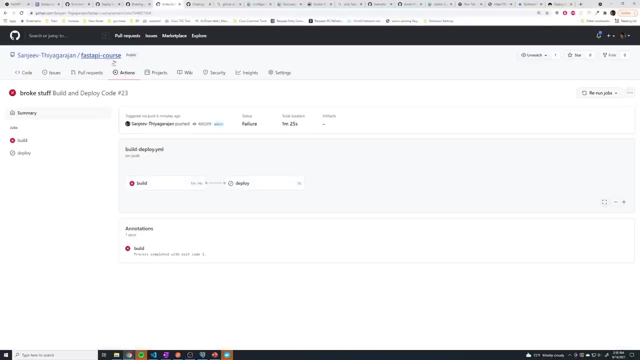 Let's fix this code real quick. And was a test posts And we'll change that back to a 200.. Don't need those notes anymore And now let's push out those changes once more. Alright, and we'll go back to GitHub again. 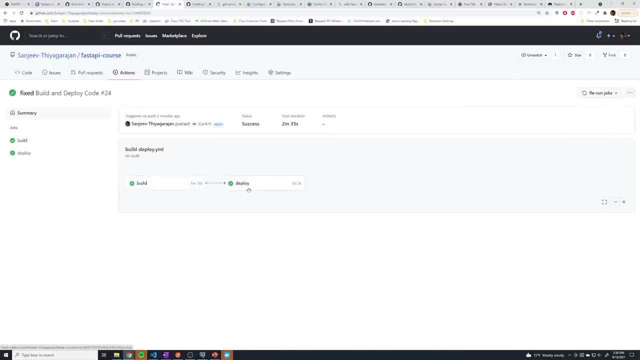 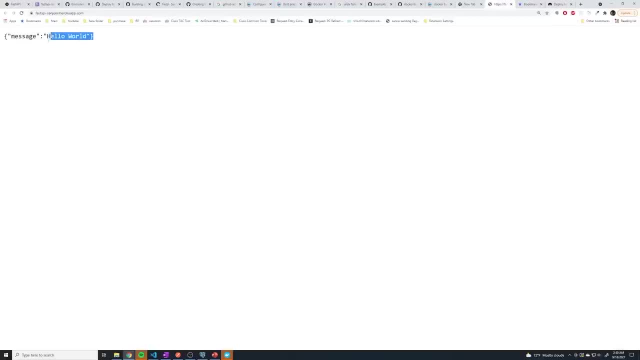 And let's go back to Actions And let's take a look And we can see the last one did get deployed, built and deployed successfully. So if I go to Heroku refresh this, we should see that this gets updated. just fine. 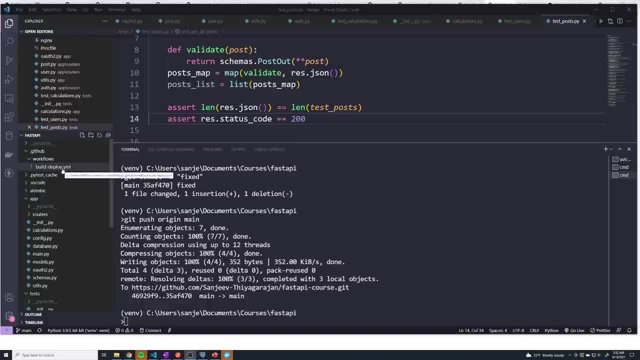 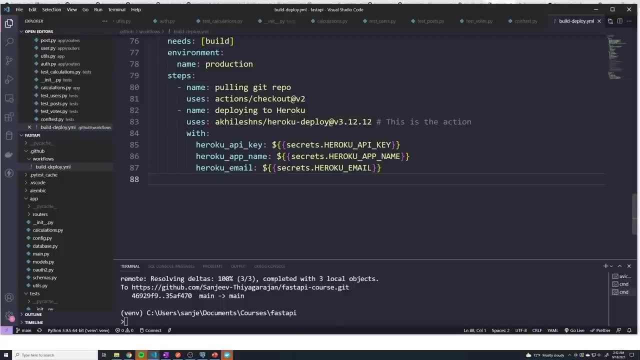 Alright, so now that we can deploy our updates to Heroku, let's take a look at how we can deploy our updates to our Ubuntu server. So, once again, it's just a matter of figuring out what exactly are the commands that we would need to run to update our production environment. 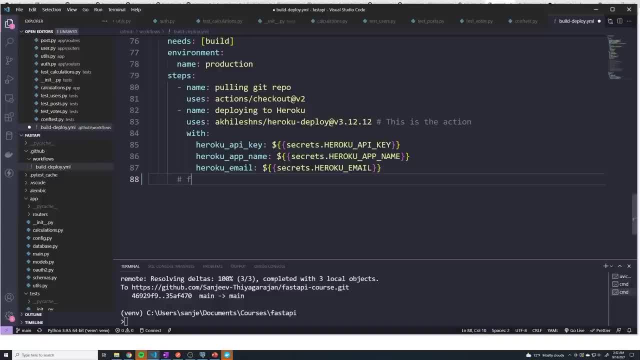 So there's gonna be a couple things. The first thing is, first of all, we would have to log into our Ubuntu server And then, once we log in- when I say log into our Ubuntu server, I mean like SSH to it. 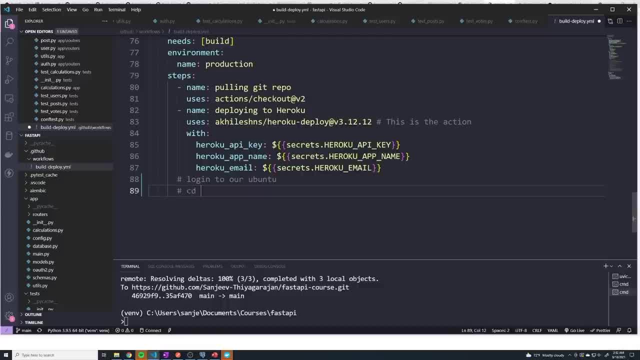 we would then have to move into our slash app slash source directory And then we would run a git pull so that we can pull the latest code, and then we'd have to do a systemctl restart API. So how exactly do we do all of this? 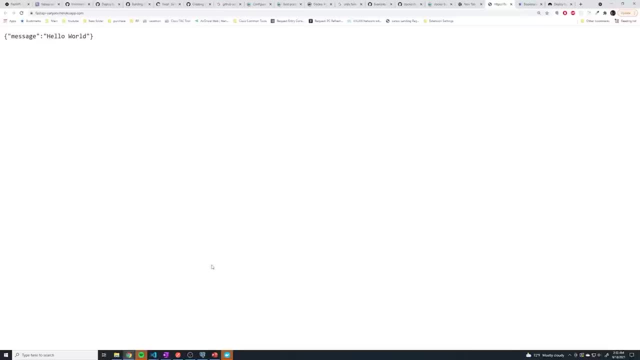 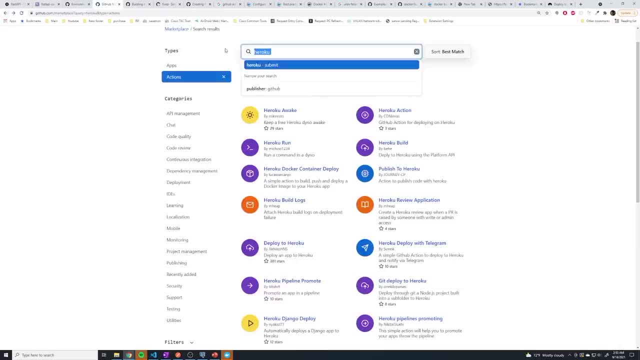 How do we log into our Ubuntu server? How do we SSH? How do we SSH to it? Well, there's a. there's a really nice built in action. I can find the marketplace again And I believe it's called SSH dash action. 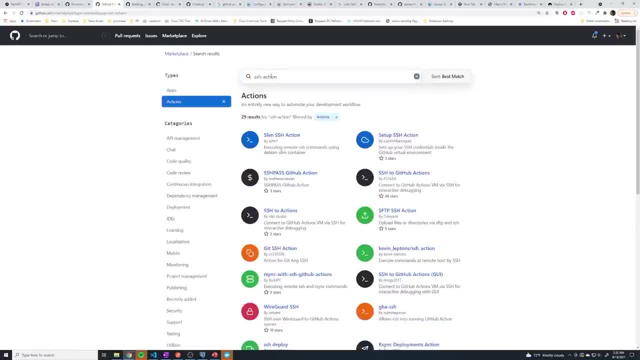 And I don't think that's- I can't find it in here- the one I used, But it's by Apple boy And I'll just do Apple boy SSH, So search for that. That's there we go. This is the one we want. SSH remote command. 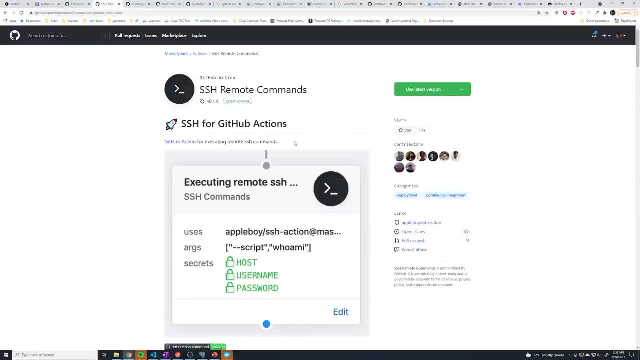 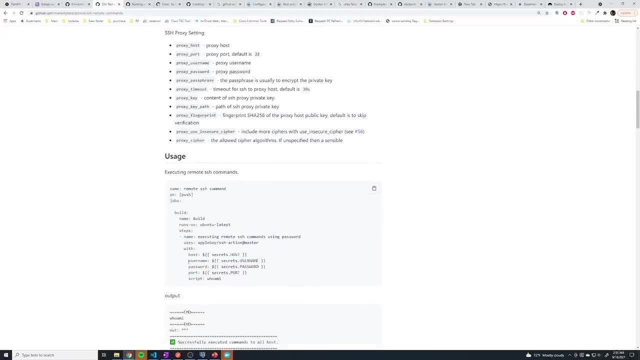 So this will allow you to run commands on a remote machine. So let's take a look at how to do this Here. they give you an example. So you have to pass in the host, which is the IP address, the username and the password. 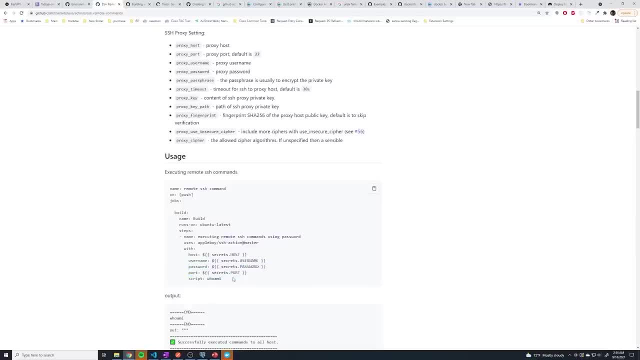 And then the SSH port is optional, but I think it should default to to port 22,, which is the one that's running on our Ubuntu server. So we don't actually have to define that, But that's all we really need. And then the script is going to be the commands that we want to run on the remote machine. 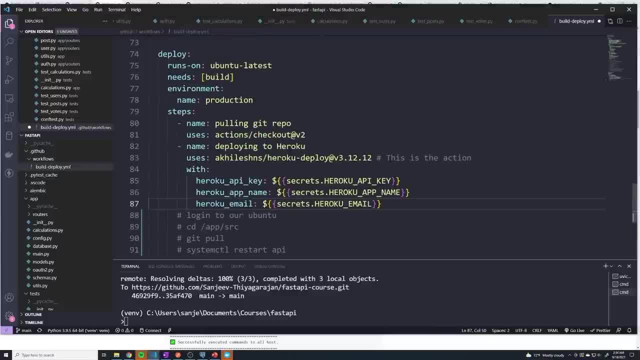 So let's set this up And I'll do that. Okay, So I'm going to go down to here And I'll say: name deploy to Ubuntu server And we're gonna say: uses Apple boy, slash SSH, dash action at master. 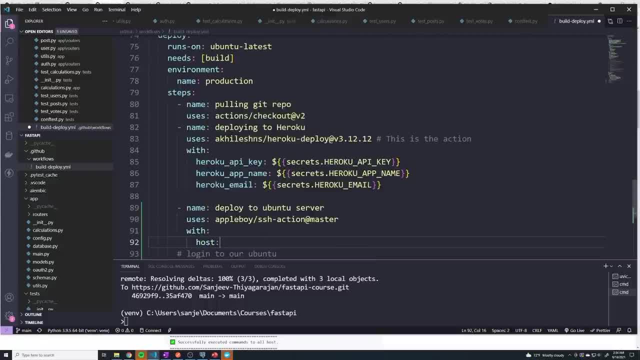 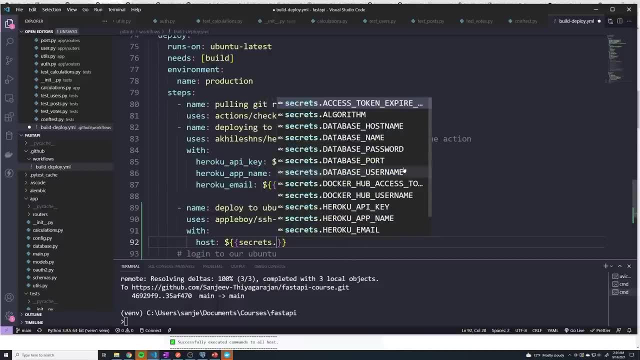 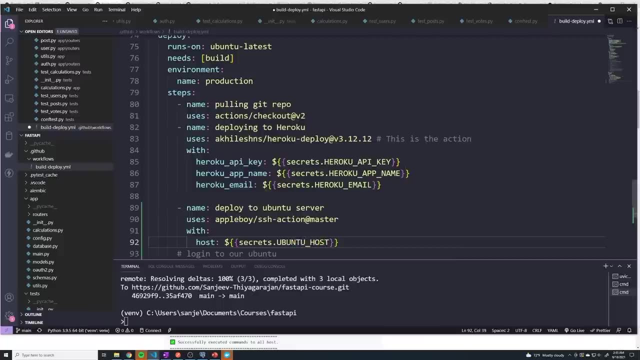 And then, with the first, we have to provide a host, And I'm going to store this in a secret and we'll call this Okay. So what do you think we should call this about? a bun to underscore host? Actually, we'll call this prod host. 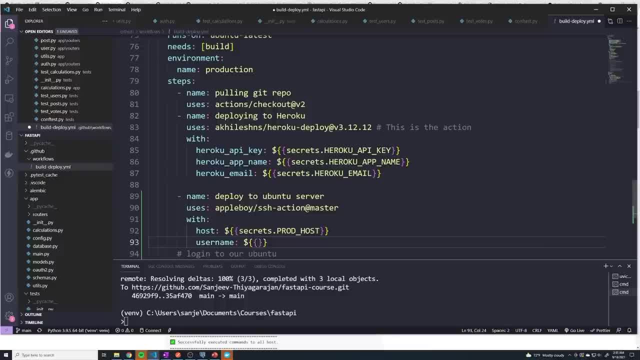 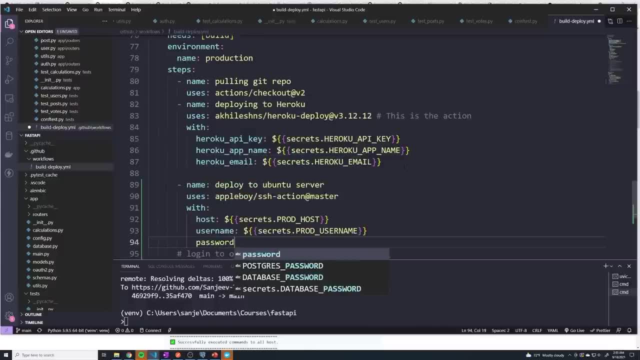 And then username: Same thing. We're gonna store this in a secret, So we'll do secrets dot prod username And then password, once again in another secret, And I'll call this prod Password. All right, then we have to provide the commands that we want to run. 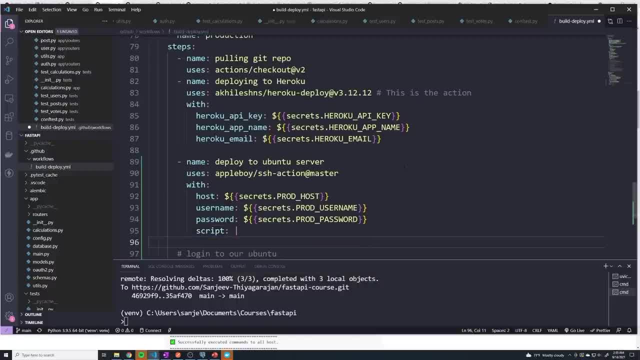 And so, since we're going to use more than one command, we're going to do the little pipe symbol And then here we just list out the command. So the first thing that we want to do is we need to move into our app directory. 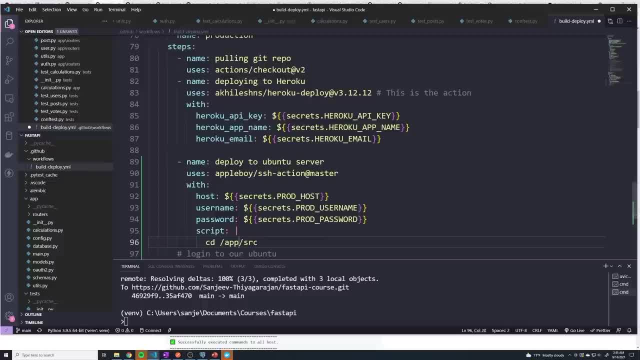 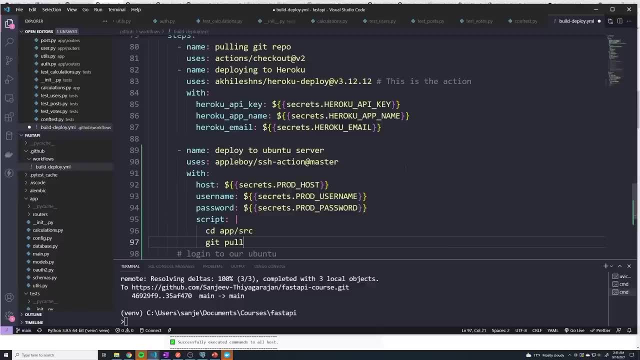 So it's going to be the app slash source And make sure there is no front slash. that's going to break things. Then we want to do a git pull. Now, This is where it might get a little interesting. I'm going to do it the wrong way first. 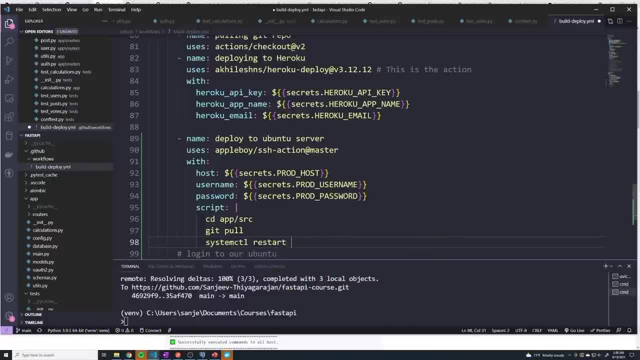 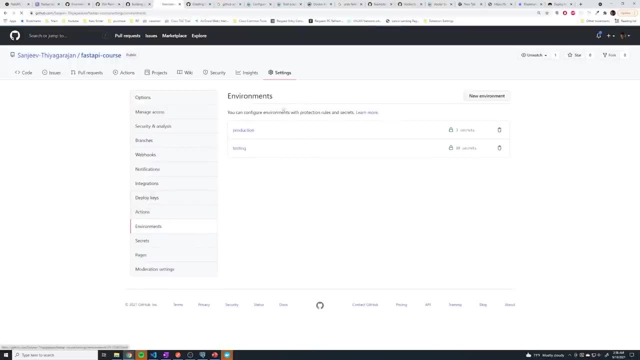 So we do a system CTL restart API, but we do need pseudo privilege. So we'll do pseudo restart API, or whatever you call it yours. And so let's define these secrets real quick And we'll go into the environments and then we'll go to our production environment. 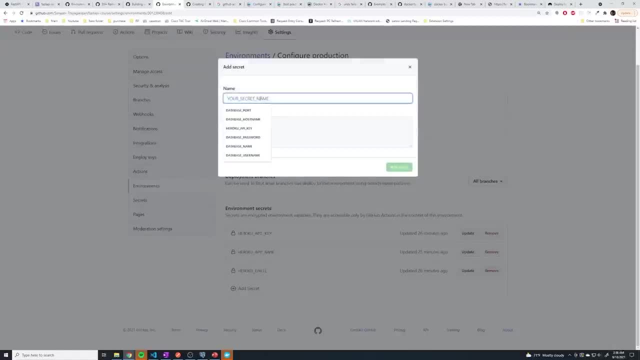 And so just go ahead and just create them here, All right, and then we're going to put in our password. I'm not going to show this one to you guys, So I'm just going to pause the video and then add it myself. 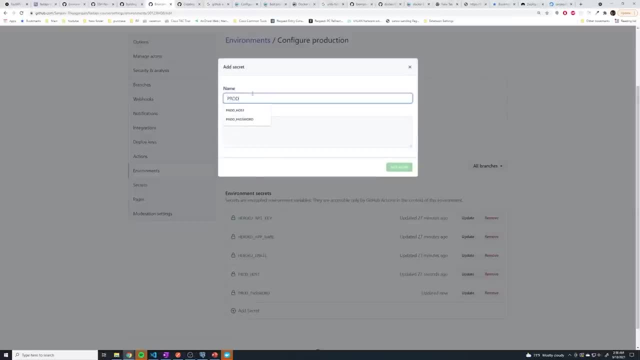 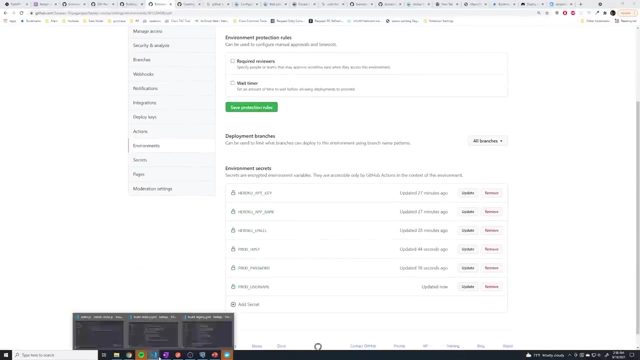 And then, finally, we need the, the username, And I believe I called it. I'm sorry, I'm sorry, I'm sorry, It's mine, Just Sanjeev. I think that should work, hopefully. And so now we've got all of our secrets. 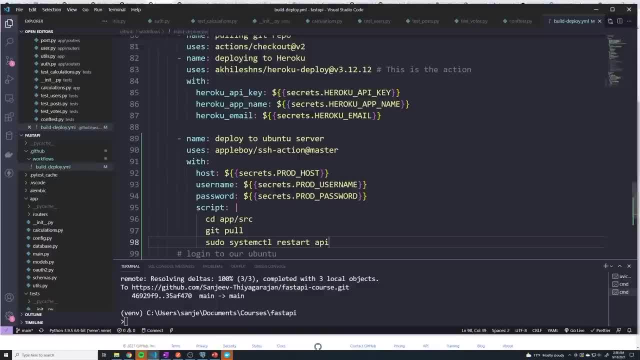 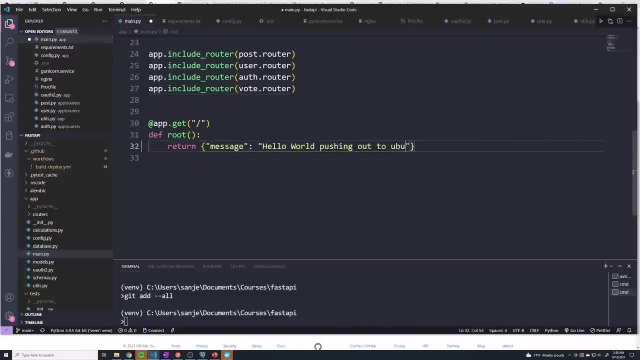 And I think we should be good to go prod host username password. Let's try this. Actually, before we do that, I'm going to make one more change to the codes that we can actually see the changes, And so this is pushing out to Ubuntu. 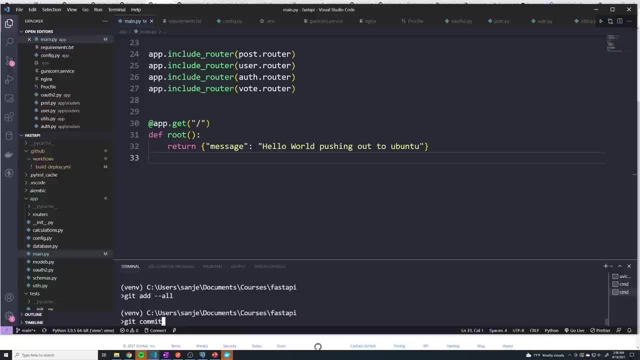 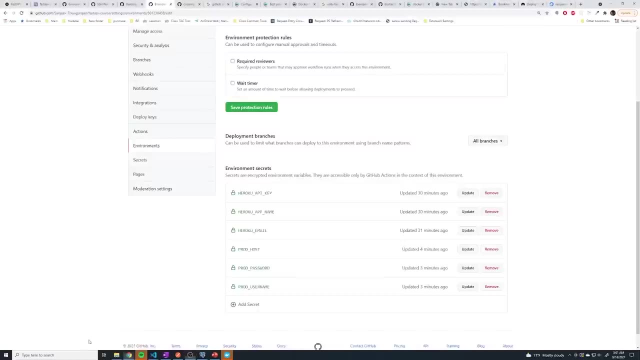 And we're going to have to do a git add once again, And then git commit, And then git push origin main. All right, and let's go back now. Let's check on our actions And it looks like it's still running. 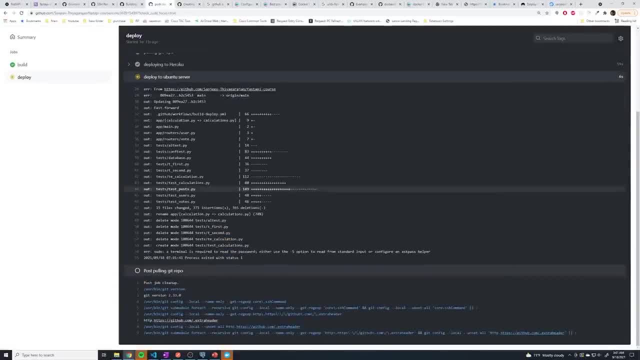 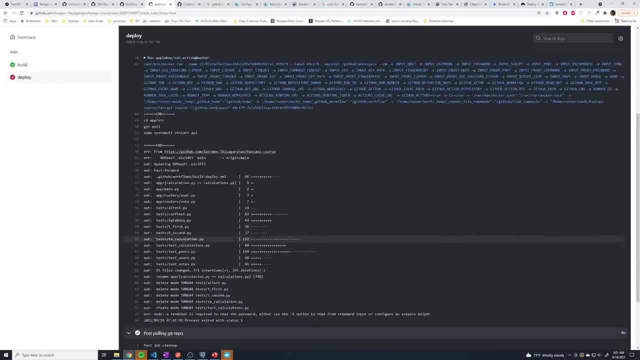 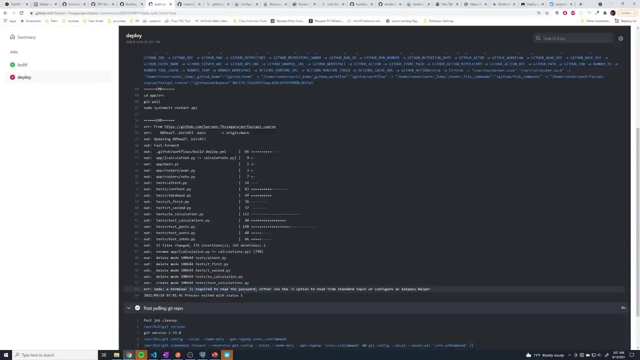 So it's in the deploy phase And it looks like it's connecting up and it looks like it just finished And it failed. So what exactly happened here? If we take a look at the logs, it says sudo- a terminal is required to read the password. 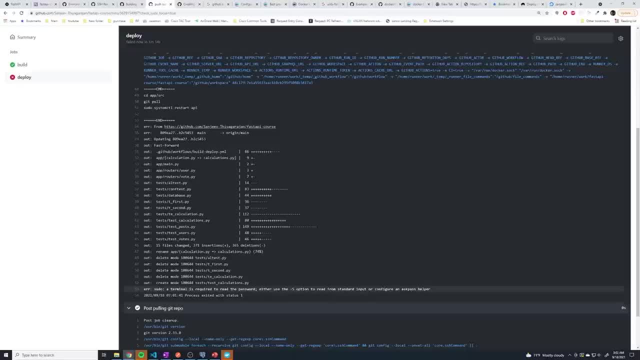 So it's basically saying that when you run the sudo command, you know you get the prompt so that you can input the sudo password. And since this is all through a remote SSH connection, that's not really an option, So we have to pass in the dash s option the dash s flag. 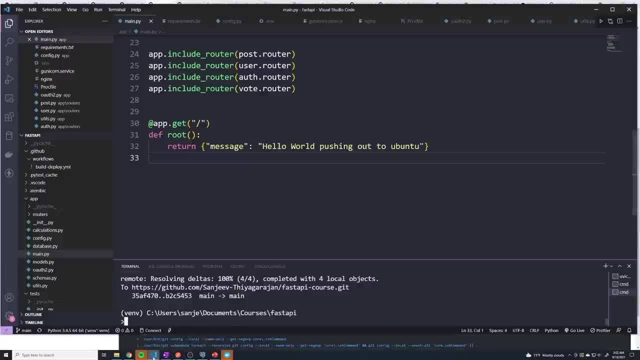 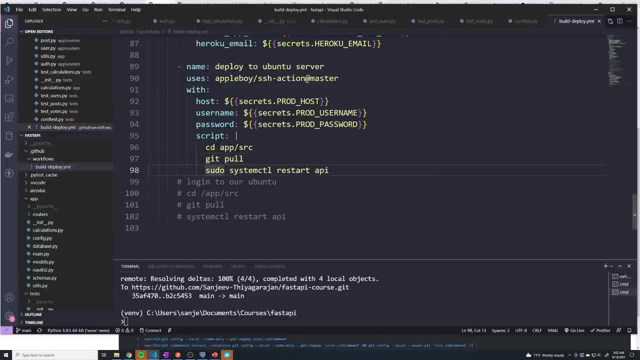 And so the way we actually define this is going to be actually pretty interesting, But Let's see where's my file. So, to use the dash s flag, what we're going to do is we're going to say echo, And then we're going to echo the password, our sudo password. 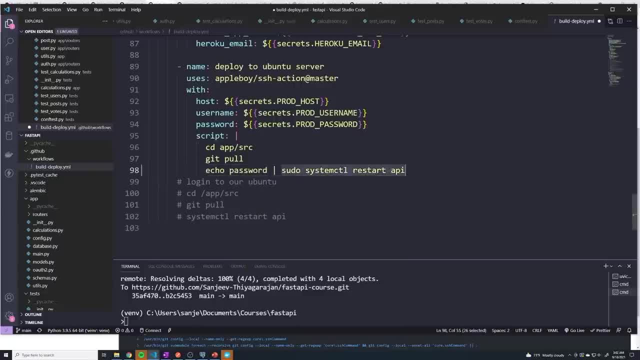 And then we pipe into the next command and we do sudo, dash s. So the dash s means that we're going to accept what the password as an argument, essentially- And this pipe command. What it's doing is We run echo and then, whatever our password is, 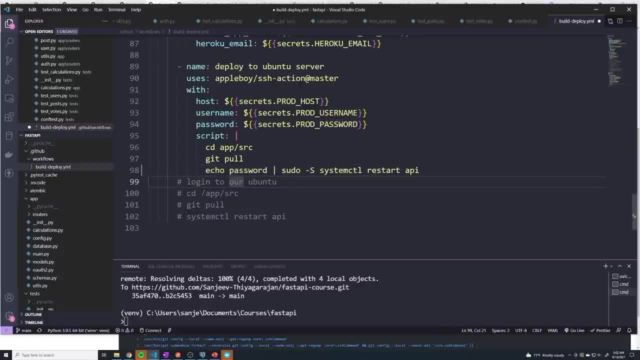 So this we actually replace with the actual password And it's going to pass that into the input of this command. So it's going to pass it into the dash s flag essentially. So that's how you do this with the one line command. 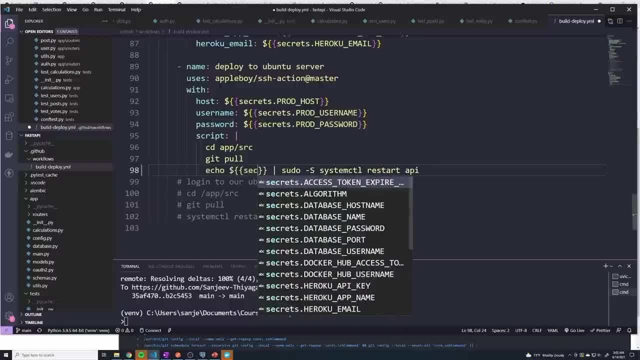 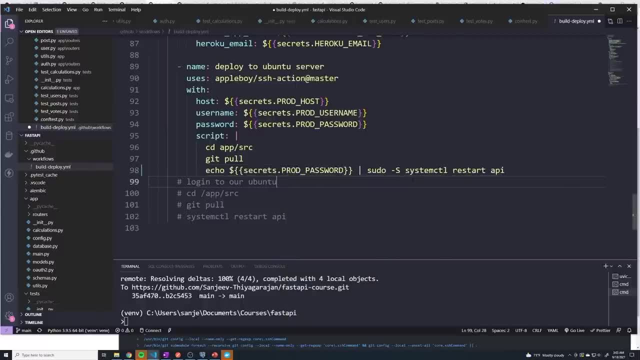 Here we're just going to pass our same environment variable, So we'll do secrets, dot prod password, And I think that should fix it actually. So D'All, git commit m, password fix and a git push Okay. So let's go back to our actions.